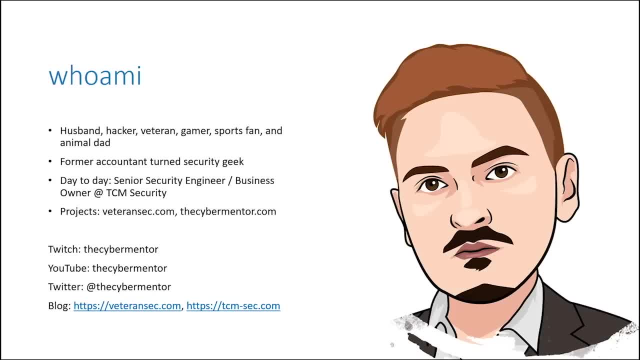 am also a penetration tester. I own my own pen test company. Before that I was a penetration tester and a senior penetration tester. I do live streaming YouTube content and etc. You can find me on Twitch at the cyber mentor. You can find me on YouTube at the cyber mentor and on Twitter at the. 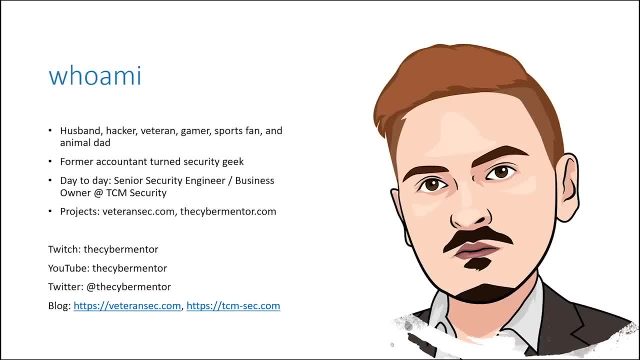 cyber mentor. If you want to check out some of my previous courses or anything, you can find them on those channels. You can also find it at the cyber mentorcom And if you're interested in any blog related stuff, veteran seccom or TCM dash. 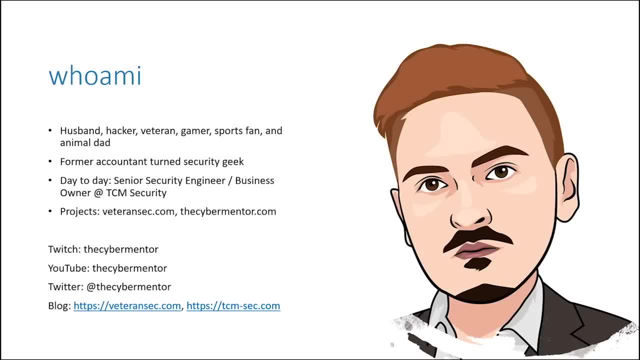 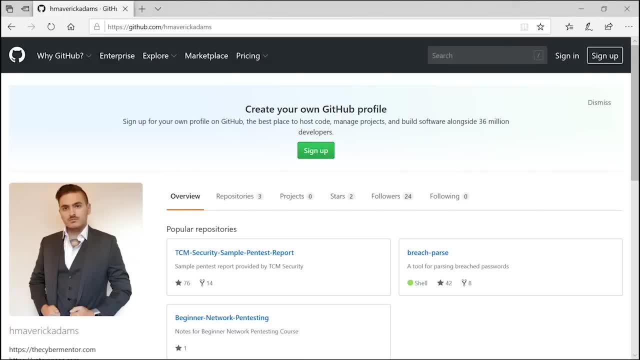 seven, So let's dive into the course and what we're going to be learning. To do that, I want to go ahead and go to my GitHub repository, And there are some reasons for this, So ignore the snazzy photo here, If you. 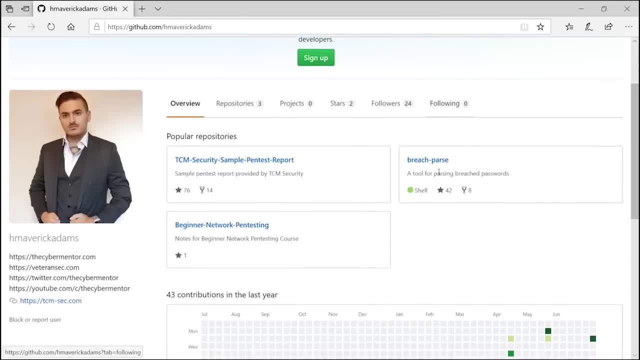 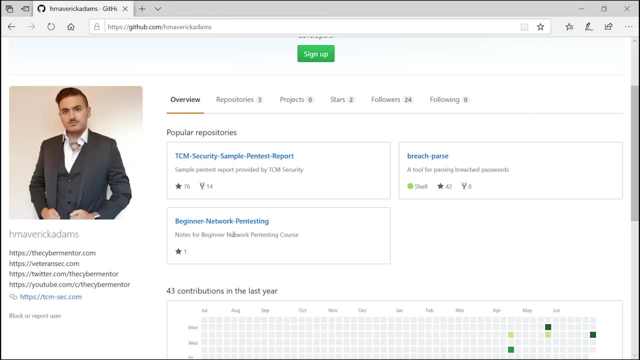 go to GitHubcom, Slash H, Maverick Adams. you can see I've got a few repositories here, So the repository we're going to be focusing on is this beginner network pen testing. There's also this breach parse and the sample pentests report. 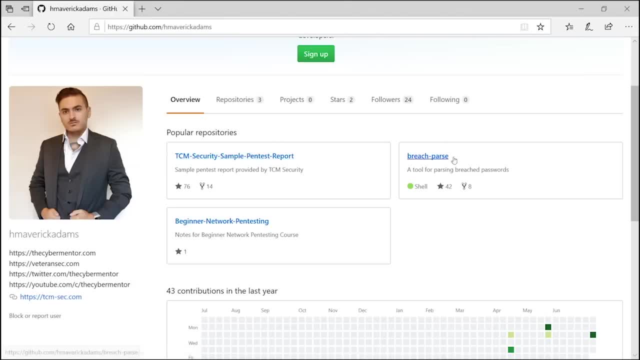 we will be using these through the course as well, So it might be useful to just notate that they're here and you'll be needing them for the course. But if you go into this beginner network pen testing, you'll see that it's going to be broken down by weeks, week one through 11.. And if you click on 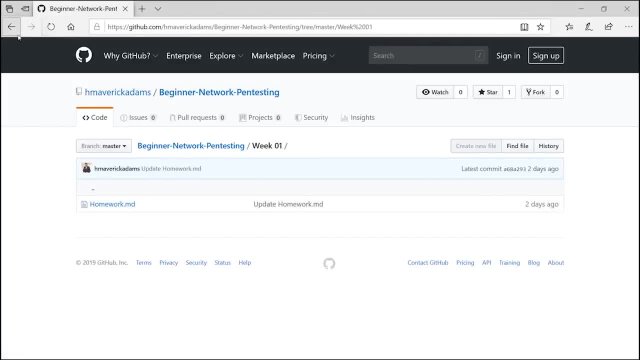 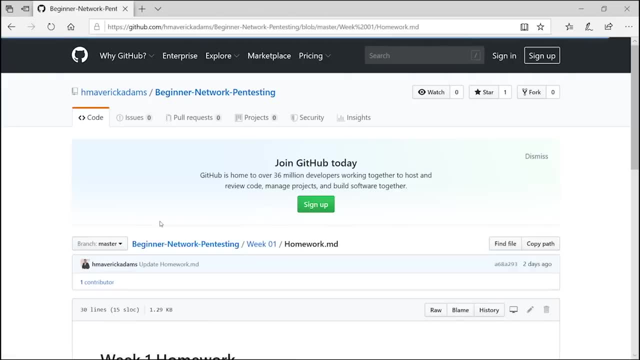 any of the weeks there's going to be homework built into it, So I recommend going in. if it's week one, you're watching the first lesson, go ahead and just click week one. click on the homework And you'll see the email that I sent out during the week that this actually occurred. 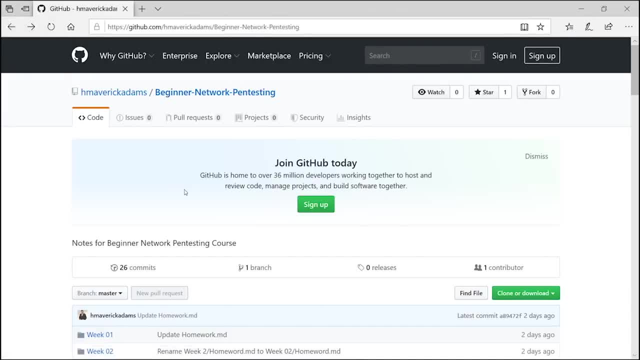 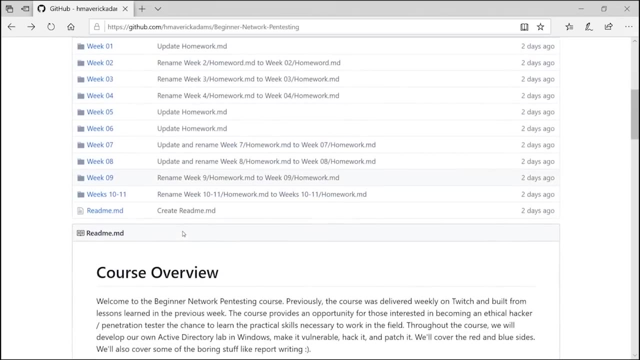 So this course was originally recorded on Twitch And each video was anywhere from two to four hours long. What I've done is condense the course down into material that is relevant and isn't like AMA or questions from the chat, since it was live streamed And if you come down here and we can 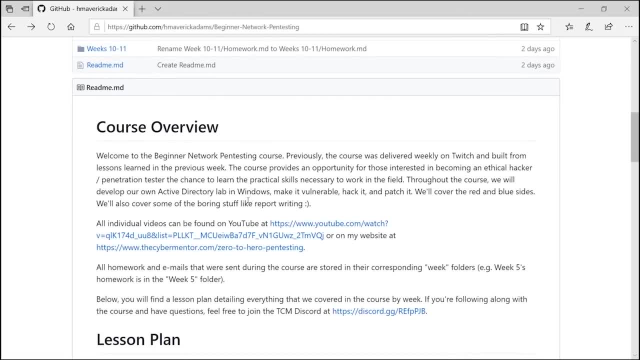 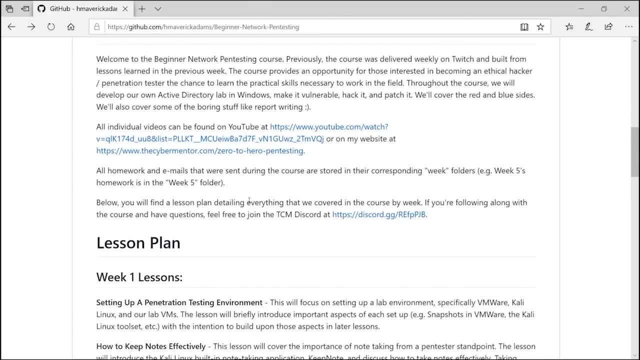 actually talk about what the course is. it is a beginner penetration testing course, So this is for people who have never done penetration testing before. you might be weak in Linux, you might be weak in Python And I'm going to take you from. originally was called: 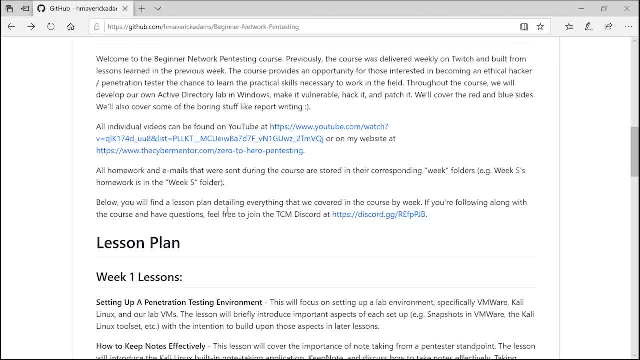 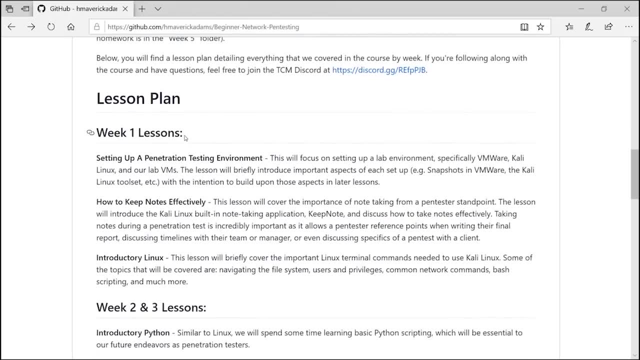 zero to hero. I'm going to take you from zero to hero and teach you everything I know about beginner network pen testing. So if we look at the lesson plan here- and I'm going to put it all down below- in the description you'll have the information for each week or each episode. 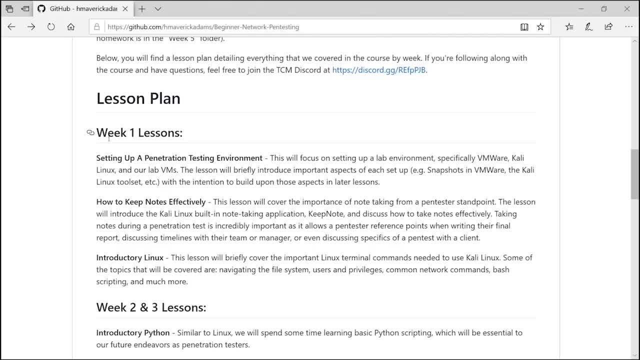 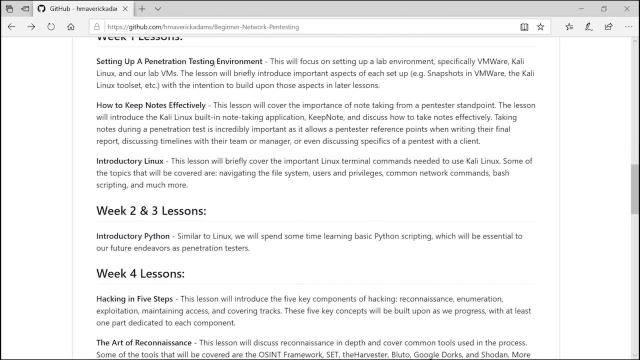 Or part with a timeline attached to it So you can just click and skip ahead if there's a lesson that you say: Hey, I already know that, But you can come here for the lessons. Lesson one is going to be setting up our pen test environment. we'll talk about note keeping tools and Linux Lesson. 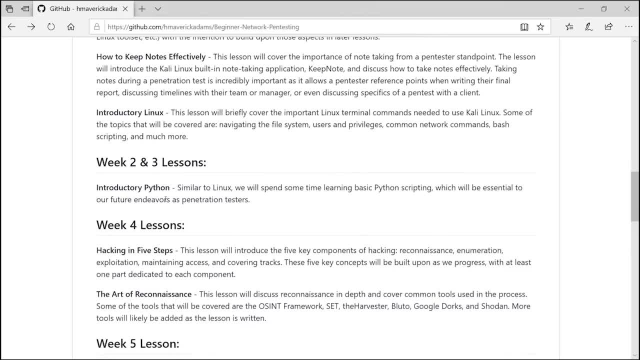 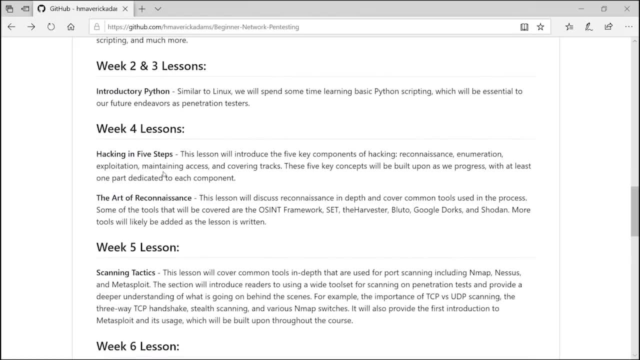 two is going to be talking about Python. Lesson three is also about Python. we just build from the previous week and then we start building out scripts and tools. Week four: we're going to talk about passive OSINT And the five: we're going to be talking about Python. we're going to talk about 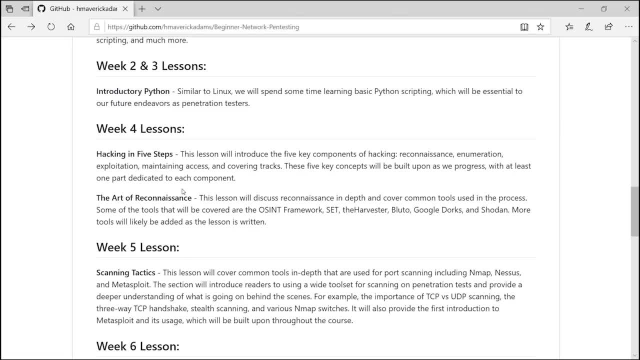 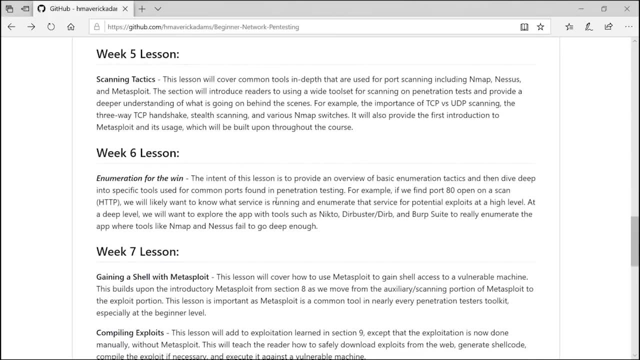 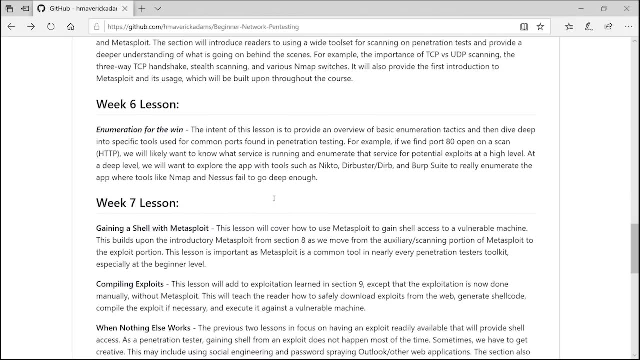 five stages of hacking. So we'll- we'll do some OSINT on Tesla from a bug bounty program and just see what kind of information we can find. And then we start diving in from week 567.. We we start learning how to scan, how to exploit, how to gain shells. we'll talk about things that we do if we 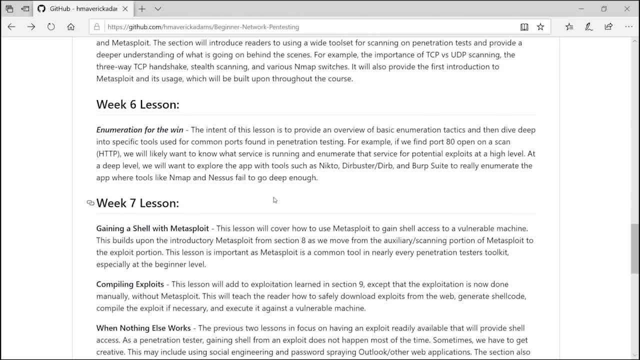 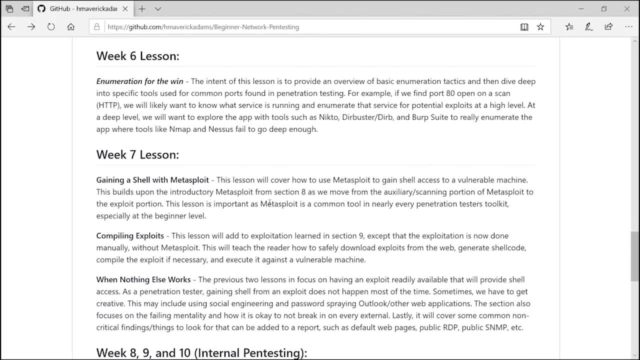 don't find anything like, if we don't find any exploits or vulnerabilities, maybe we can do some things like credential stuffing or password spraying. So we'll talk about what those tactics are and how they work, And then we're going to talk about some of the things that we're going to. 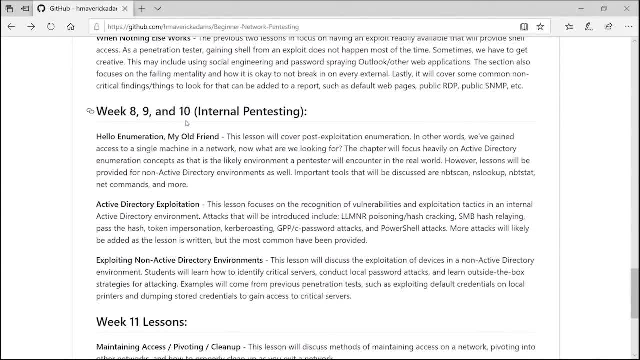 learn how we can use them. And then we go in for week 8910 into internal pen testing, So actually build out an Active Directory lab And then we'll exploit that Active Directory lab. So we'll learn a bunch of new things and new attacks, LLM and our poisoning with hash cracking SMB relay pass the. 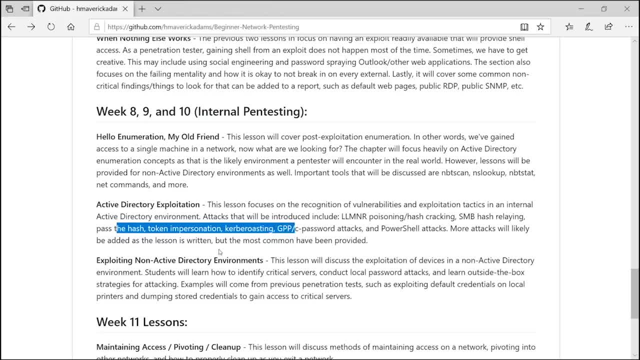 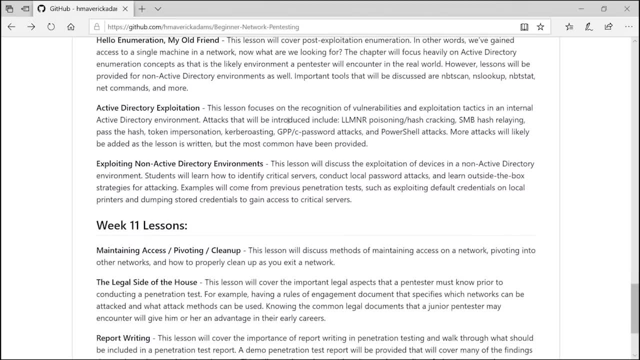 hash token, impersonation, Kerber roasting, etc. There's a lot of attacks in here that we're going to be learning. And then, lastly, when we're done with the Active Directory slash, internal pen testing side of things, we'll talk about the maintaining access, pivoting and cleanup that are part of the five stages of 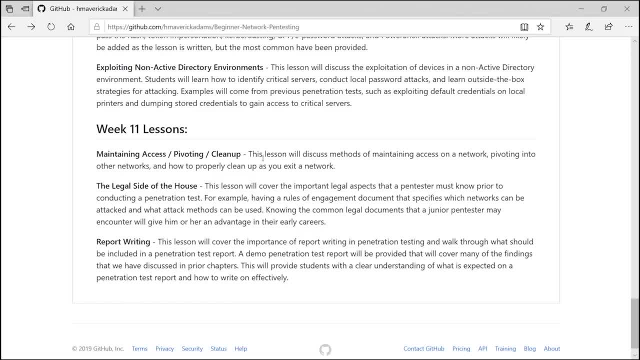 hacking. We'll talk about the legal side of the house, meaning we'll talk about what type of legal documents you might encounter, such as like a master service agreement, rules of engagement, etc. As a pen tester. From there, we'll talk about report writing. So you saw that sample report from. 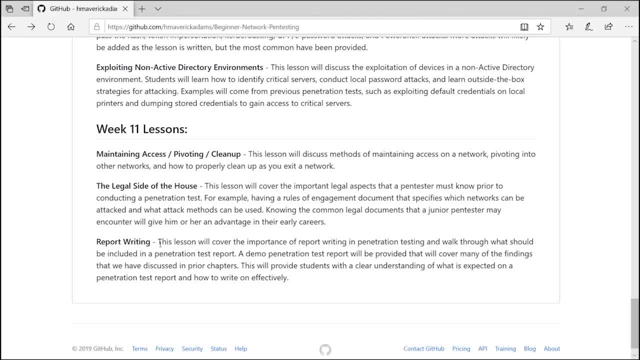 the previous page we'll cover a sample report, what it looks like and what you should be including in a pen test report. Lastly, we'll cover which is not in here. we'll cover some career advice and my recommendations for finding a job. So if you take this from week one to week 11, you start with basic Linux, you move all. 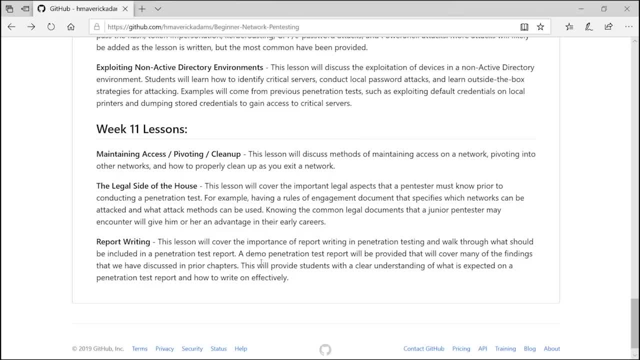 the way through. you are doing external, internal pen testing And by the end of it you're not only doing that, you're writing reports. you've got career advice. you understand some of the legal side of the house. So again, I just want to notate that as you go through, I will mention homework in 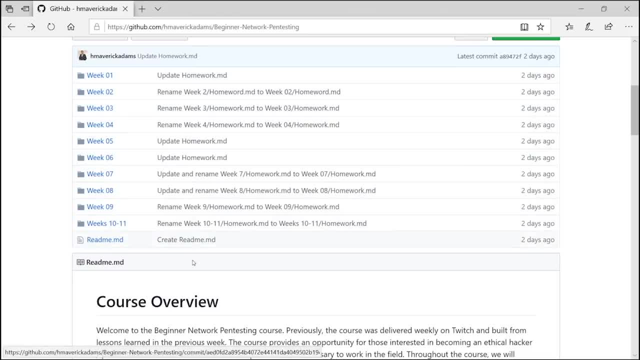 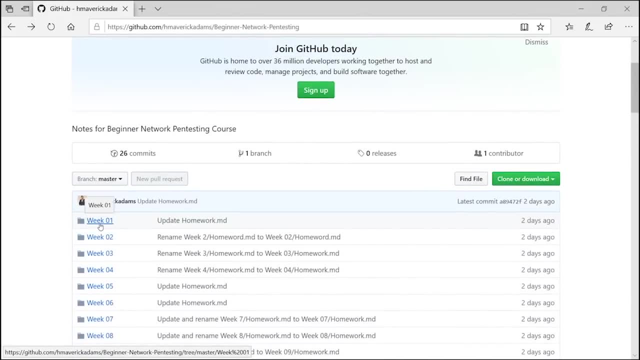 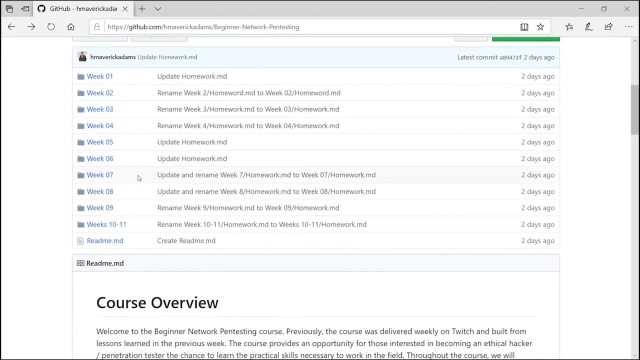 the course. So if you hear me mentioning homework, this homework is found in the week here. So if you just tie in week one lesson, come in here, click on the week one, look at the homework and then go ahead and get started with the, the materials. So you might get a little loss if you don't look at the. 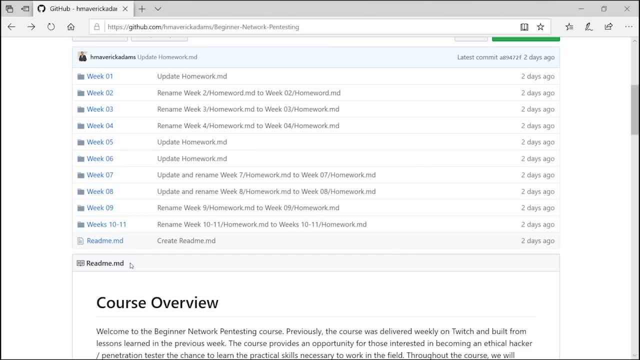 homework. But, with that being said, I want to dive right in. If you enjoy this course, you enjoy this video. please do consider sharing it with a friend. hit that like button, that subscribe button. Word of mouth is the way I've been growing. And then, if you want to check me out of 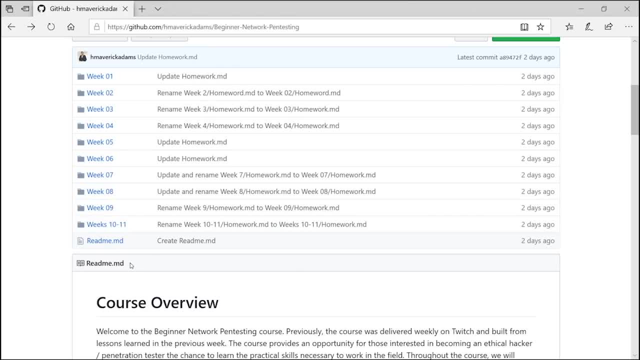 course, YouTube is great. You can also check me out on Twitch. we do live stream pretty much every Wednesday night. So, again, my handle is the cyber mentor And I really, really hope you enjoy this course. So let's go ahead and get started. 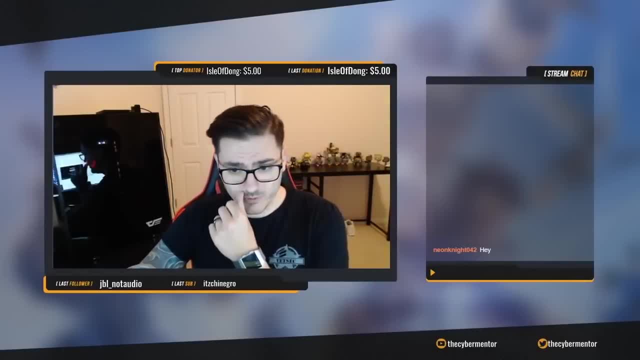 All right, guys, it's eight o'clock, we're gonna get rolling right away. So I sent out an announcement Via email and I realized that many of you aren't on the email list quite yet, So I'm going to go ahead. 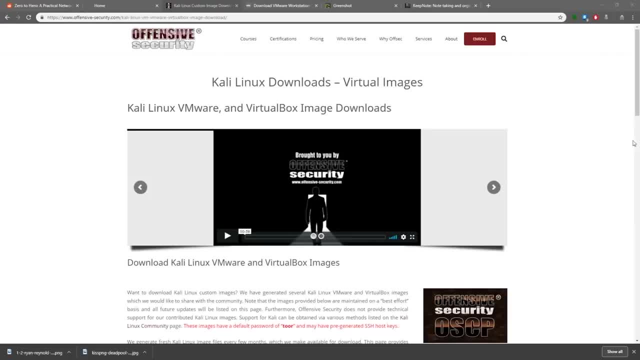 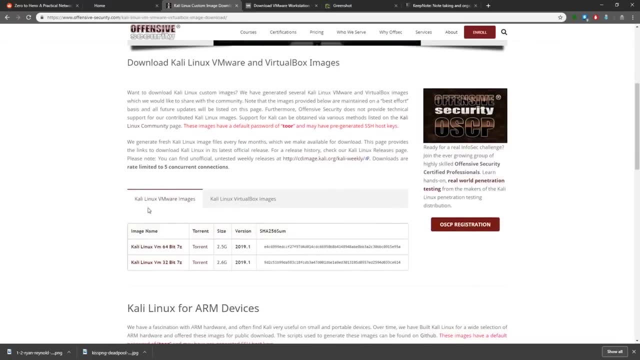 and just share my screen. So a couple things we're going to need for tonight- And these are kind of on the large side of downloads, If you haven't downloaded already- is the Kali Linux custom VM. So if you're going to be using VMware or VirtualBox, it has a tab for each. I'm going to be 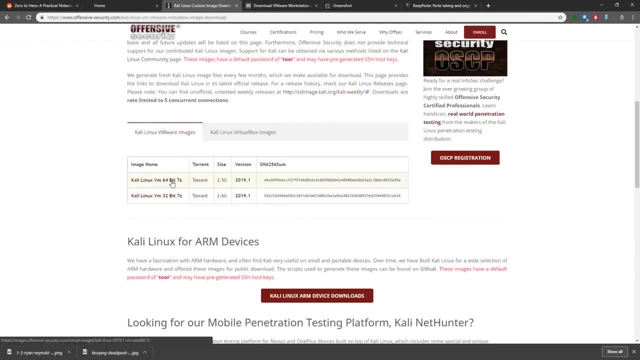 using VMware throughout the course. So go ahead and just click the link here to download the 64 bit And we're going to go with that. It's 2.5 gigs, I think, it's like nine or 10 extracted, So we're going to go ahead and use that one. You'll also need 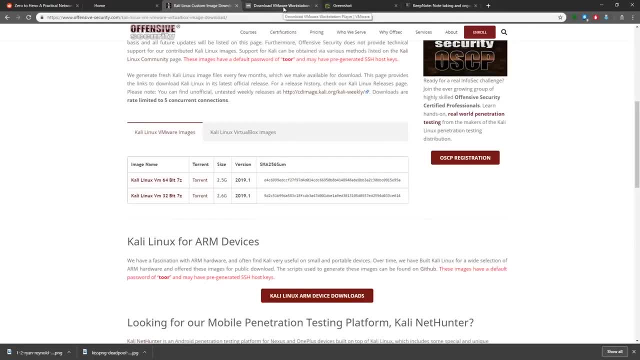 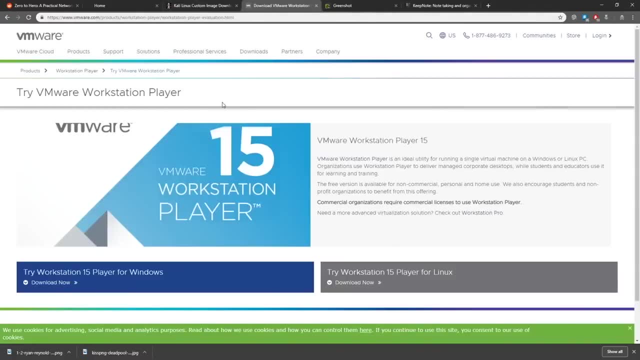 VMware. If you have VMware Pro, great. I'm going to show you how to run on VMware Workstation tonight. Workstation player. I should say So if you search out Workstation player, you just go ahead and say try for Windows or for Linux, depending on where you're running it, and get that. 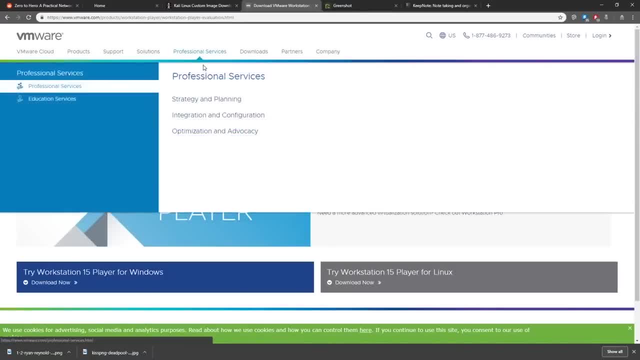 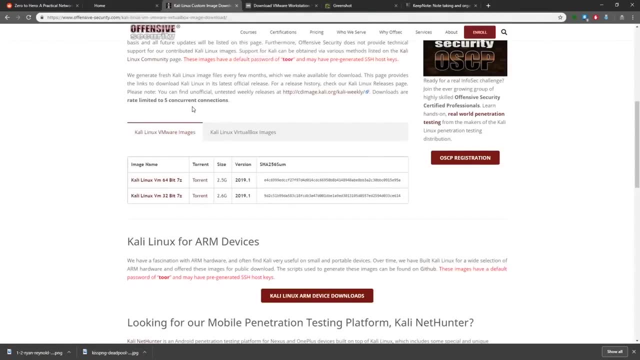 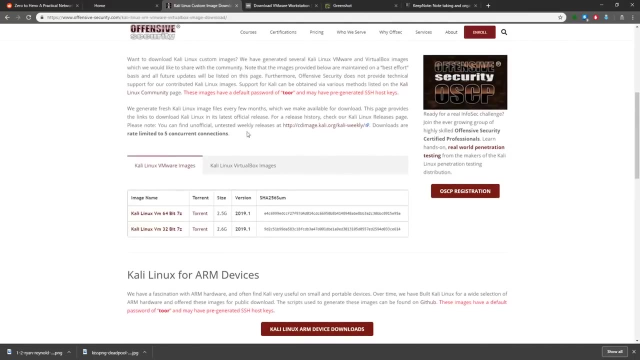 downloaded as well, So that way, when we're talking through things, you can already get this downloaded, in case you're a little bit behind. So for the Kali Linux download, I want to add in to search out custom image download for Kali on Google, Because if you go to Kali Linux, you're going to get a different page than this. you want the custom images because they're pretty easy to install. 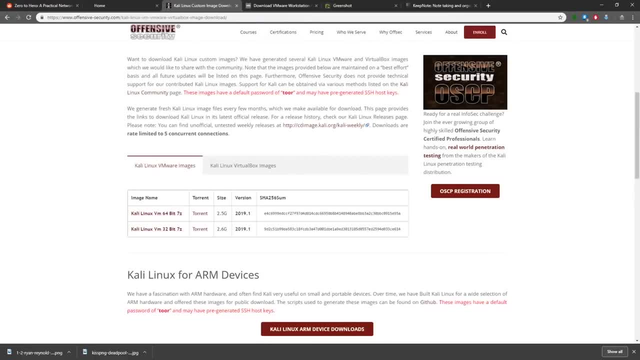 Hey, Red Finale, shalom, shalom. All right, so we're going to go into this just a little bit of PowerPoint. I swear we're not going to do death by PowerPoint, We're just going to do a quick. 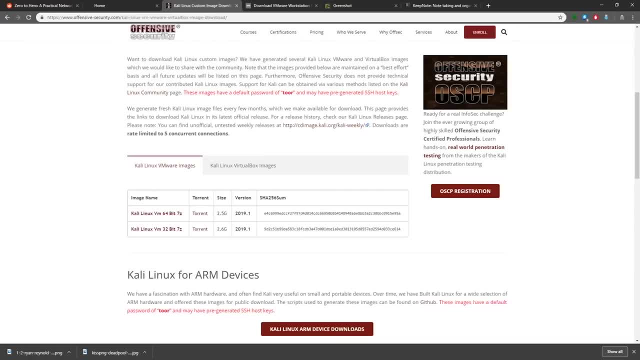 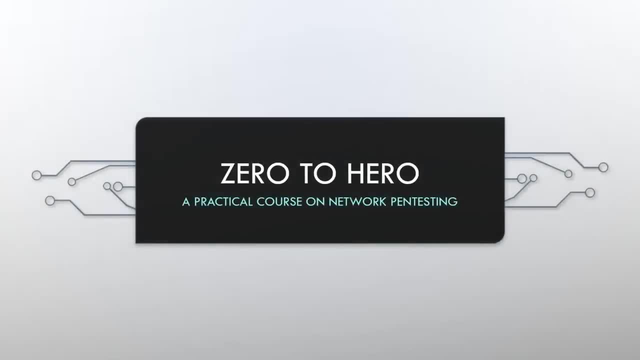 overview and then we're going to get really quickly started. So, hey, hey, frog, how's it going? All right, Kali is made by offset, you are correct. All right, welcome to the zero to hero pen testing course. This is a practical course on network pen testing. So we're going to go from zero, hopefully, to hero. So who am I? 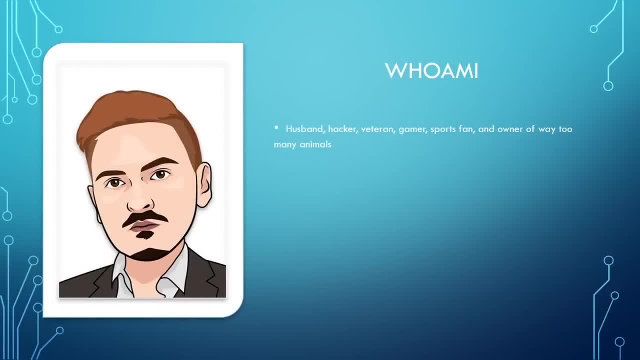 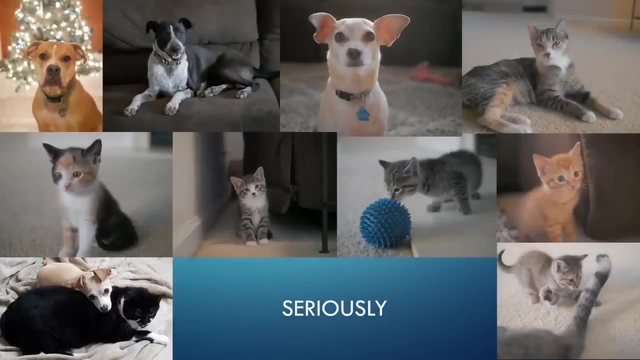 Hello, I am the cyber mentor. you may know me as Maverick, you may know me as Heath, So a few different names- but I am a husband, hacker, a military veteran, gamer, sports fan and the owner of way too many animals- And when I say way too many, I am serious. I have 10 animals in my house right now. please help me take some of these and adopt them. 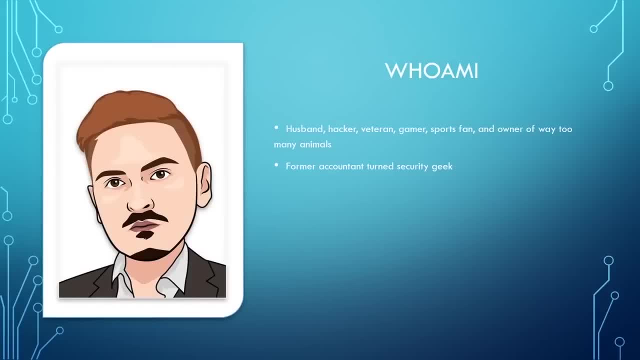 So, other than that, I'm a former accountant turned security Geek. I went my own zero to hero path in about three years, actually made it from help desk to, you know, to pen tester in two years. So it's definitely possible. I think I'm a good advocate for zero to hero. If I can do it, anybody can do it. So way too many. Yeah, this is what happens when you, when you adopt a cat right And the cat's pregnant. Well, we didn't even adopt it, She was just stray on the street, took her away. 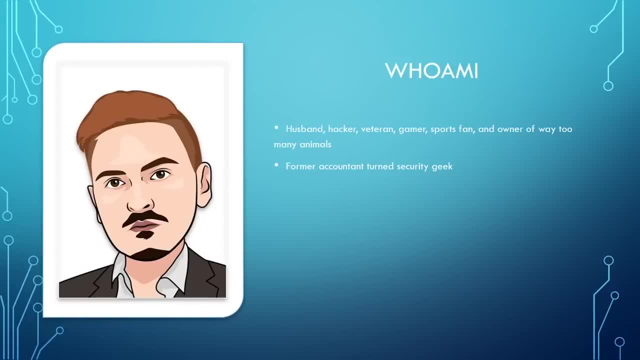 And she was pregnant And then she had kittens. So that's a quick way to add six animals to your household that you didn't even want. So yeah, pack it up guys. So my day to day at my job, I do quite a different, few different things. I wear a lot of hats. So, anywhere from internal to external- network penetration testing, web application penetration testing- we do something called sock assessments. That's kind of like a purple team, That's where you work with the blue team and you, you do a pen test. 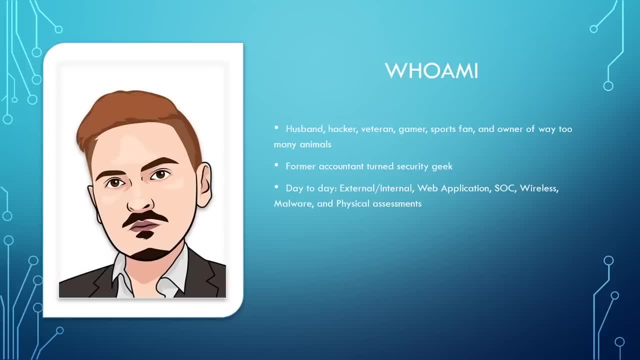 And you say, Hey, do you see what I'm doing right now? And they say yes or no, And you help them get their baselines together: Wireless assessments, malware assessments and physical assessments, which are incredibly fun if you get the opportunity to do them. 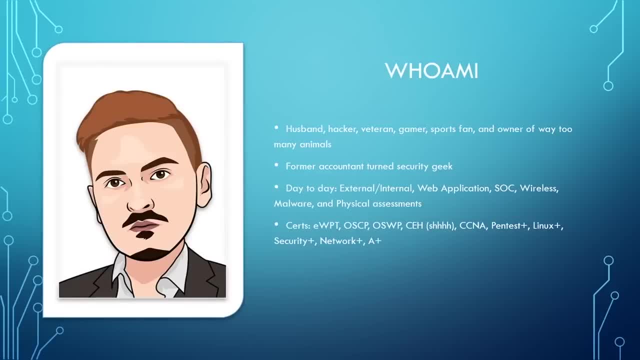 Some of the certs I have. you can read the list. don't look at the CEH. So other things I'm part of I do. I have co founded vet sec. So if you've heard of vet sec, I helped co found that about a year ago. That's for military veterans. 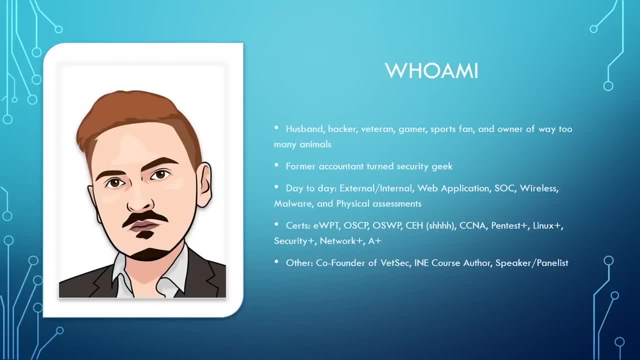 They're looking to get in cybersecurity. So if you're a military veteran of any country and you're interested in that, there is a link down below a button that says military vet question mark. So if you click on that, you can look at our Slack channel and come join us over there. I have produced a course with I&E. That was the first course I produced, So it's kind of bad in terms of quality and speaking and everything else. I've gotten much better. 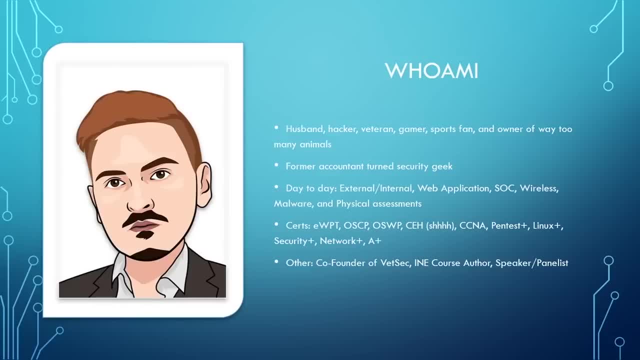 And then I am a speaker panelist. I've got a panel coming up at B-Sides this month And then next month I'm going to be speaking at CarolinaCon And hopefully a couple more cons are coming down the road, depending on what my talk is. 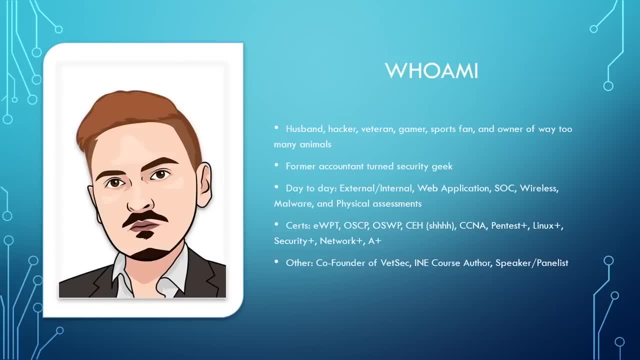 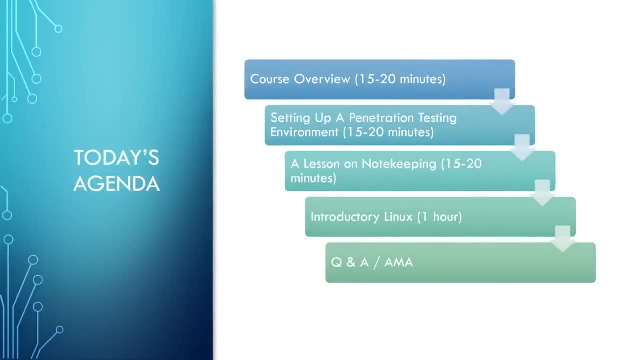 getting picked up or not. So that is a little bit about me, And we could talk about certs and AMA when we get to the AMA, kind of things. But we'll talk about that. And yeah, I just got picked up by CINAC as well. 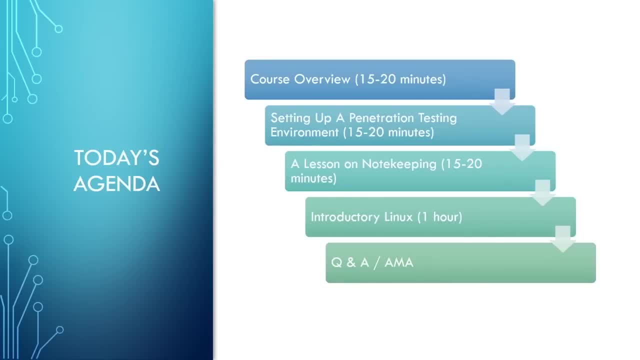 So for today's agenda, we're going to do a quick course overview. I know many of you have already seen the Reddit post, but we're just going to cover that again in case people who see this later and they're just interested in what this course. 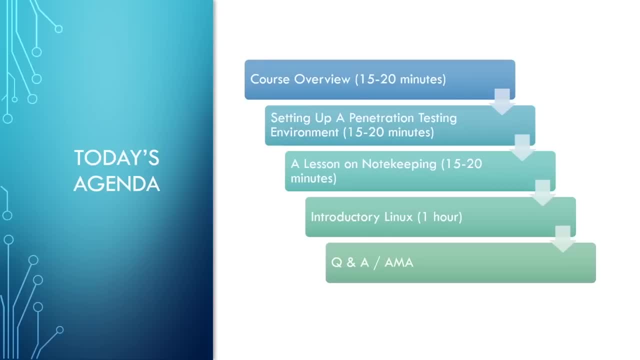 is covering. We're going to talk about that. We're going to talk about setting up a penetration testing environment. So that's why I needed you to get Kali Linux downloaded and VMware. We're going to do a lesson on notekeeping. 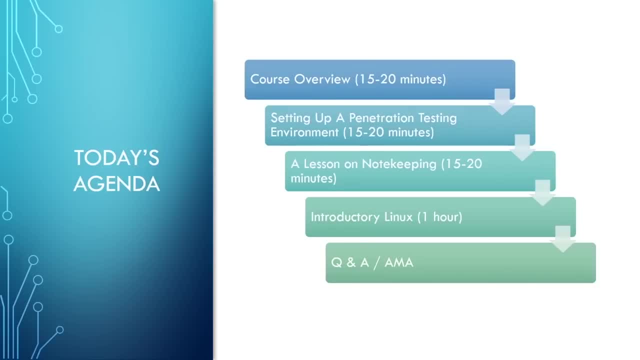 And that's where we're going to talk about our notekeeping options, including Cherry Tree for you guys who are loving Cherry Tree, And we're going to also cover introductory Linux. So we're going to cover it kind of from a pen tester's perspective. 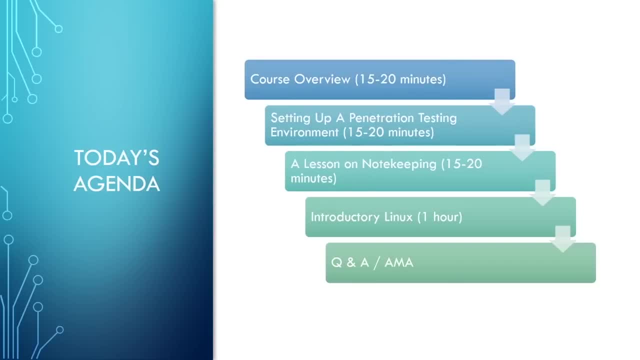 If you've never touched Linux before, this is kind of the lesson for you. If you have, you still may learn something, but it's going to be pretty basic. So, lastly, we're going to do a Q&A- AMA. 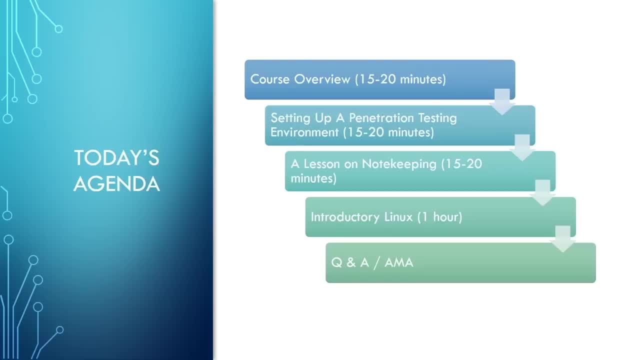 I will be here as long as you guys want me to be here and you want to talk to me. So if you've got questions I will answer them all. So just got to be patient with me and I'll kind of try to answer as I go. 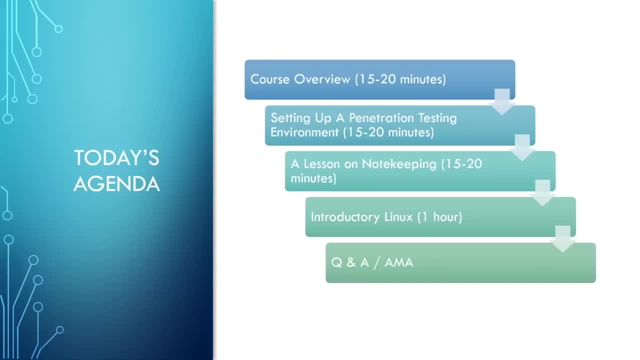 So the goal tonight is to end around 10 o'clock my time. It's 8 o'clock right now, so it'll be pretty quick pace, but I'll definitely slow it down so you guys can take notes and ask questions as well. on topic. 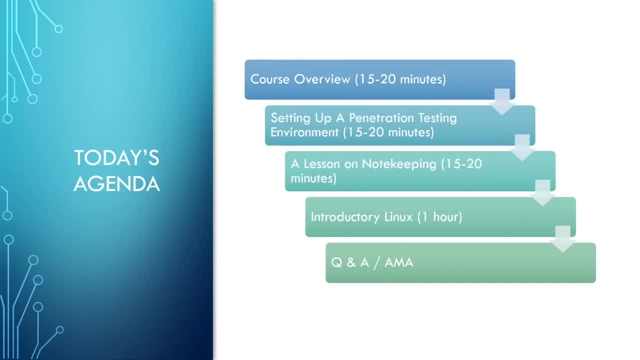 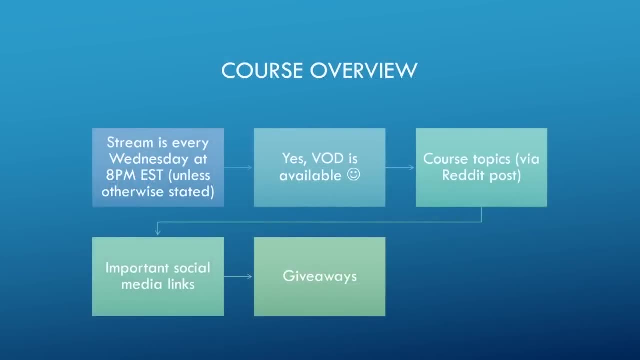 Thank you for the sub JDelta. I appreciate that. Okay, so let's talk about the course overview. So the stream is every Wednesday at 8 pm Eastern time. unless otherwise stated, That is always going to hold true. 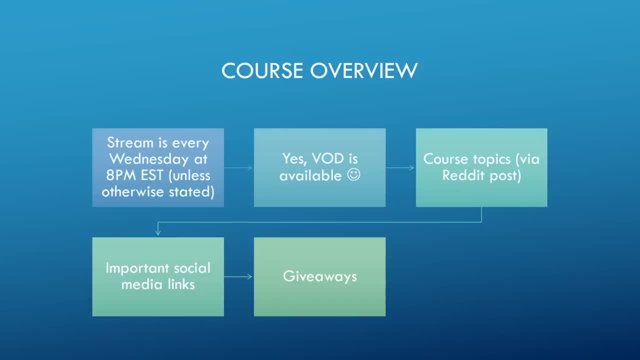 If you see something elsewhere, let me know. But that is where we're at. Uh, video on demand, It is available. So if you miss this, you're in another country, a different region can't make it. It'll be on Twitch immediately after. 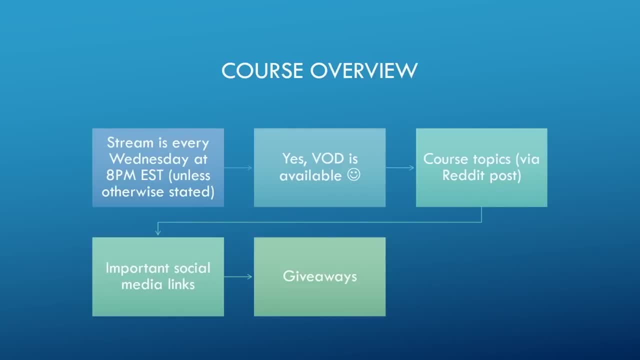 And if you can wait a day or if you need to wait a day, it's also on YouTube And I'll provide those links for you down below. So also course topics. So let's talk about the course topics. really quick, Let's go to that Reddit post that we talked about. 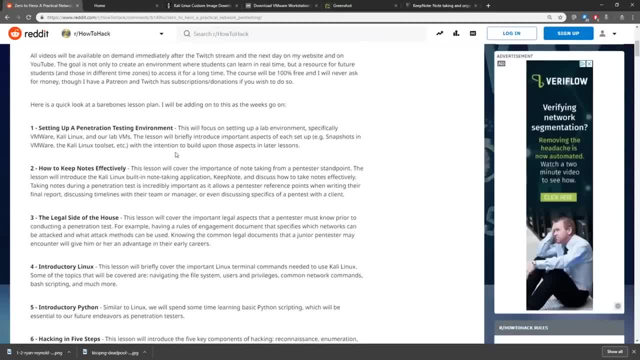 And this is just a quick overview of what we're going to be covering in this course. So I set this up to the way I would write it out, Like if I were writing a book. this is kind of how I would write it out. 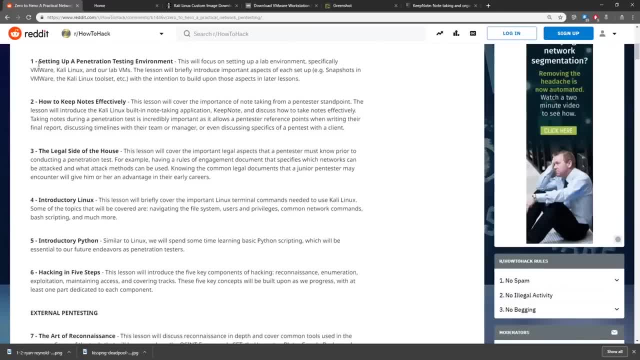 Um, but I thought that the first lesson would get to PowerPointy. if we like put all these things in here, Like, if I started getting into legal aspects, it might bore you guys to death. Um, so what we're going to be doing is I'm actually going to move this legal side of. 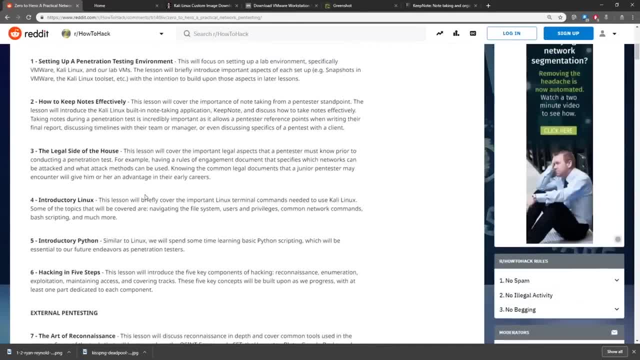 the house, probably more down towards the end when we get into um reporting. So what we're going to be doing this week is we're going to be talking again: setting up pen testing environment, how to keep notes effective, Effectively. introductory Linux. 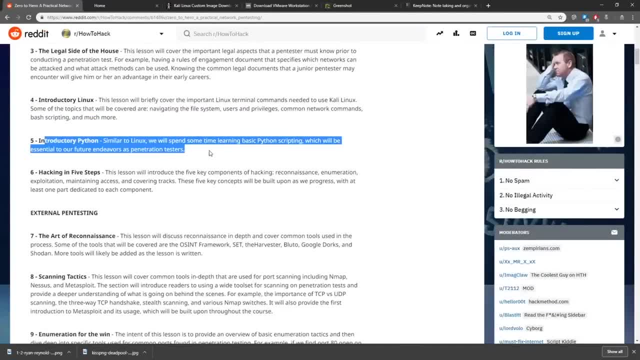 Then next week we're going to start into Python. It's going to be a uh simple Python lesson. We're not talking like getting into development level. We're talking, uh, basic scripting into maybe medium level knowledge. Uh, if it takes us more than one week, it takes us more than one week, but for the most, 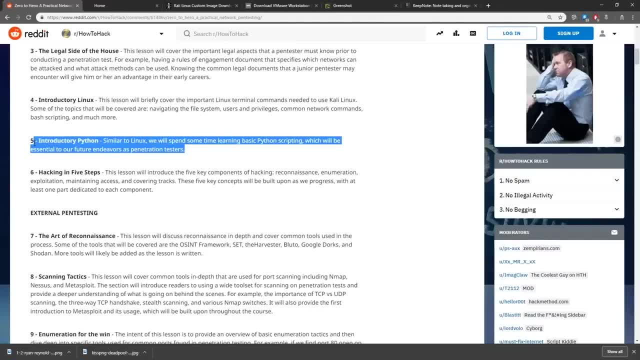 part. it should take us a week. I'm going to give you some homework on this one, So if you're not signed up for the mailing list, I'm going to show you how to do that And, uh, we'll, we'll get there. 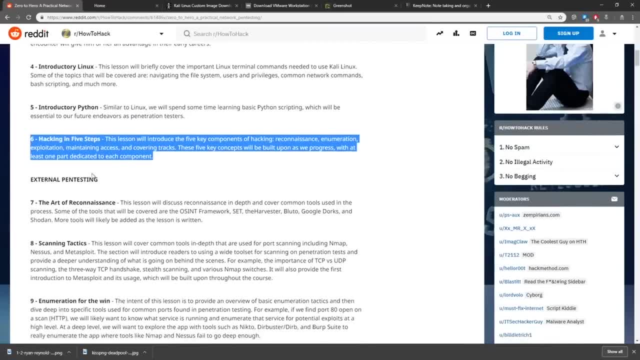 So the following week likely, we're going to be covering hacking in five steps and also covering, um, some external pen testing. So the hacking of five steps are the five steps of hacking. It's, uh, everything that you should know in terms of being a hacker, the whole process. 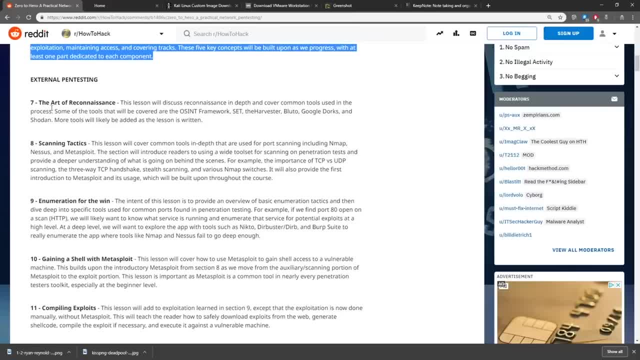 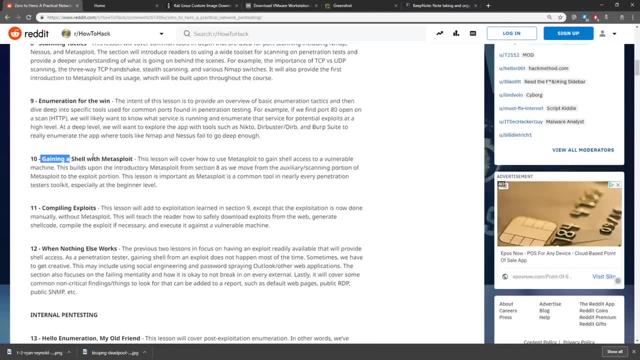 from start to finish. Um, so that's a theoretical overview, and then we're going to go in right into it. So we're going to talk about reconnaissance, scanning, enumeration. Uh, we're going to talk about using Metasploit and then compiling our own exploits. 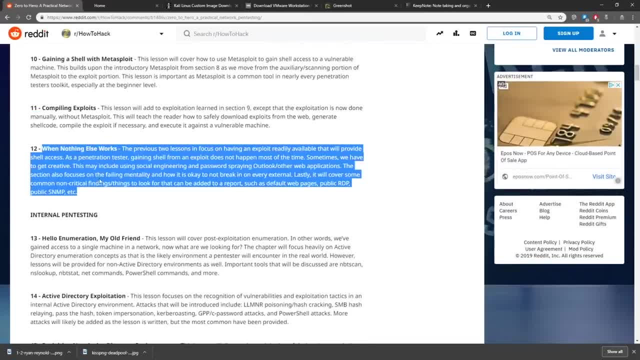 And then we're going to talk about, uh, how to do that. We're going to talk about some things that we can do when nothing else works, Um, and then on the internal side, we're going to go back to enumeration again and focus. 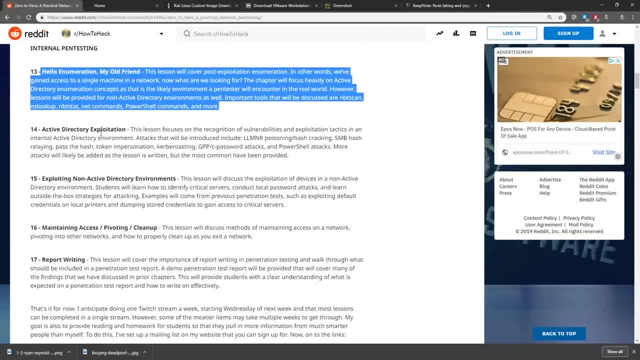 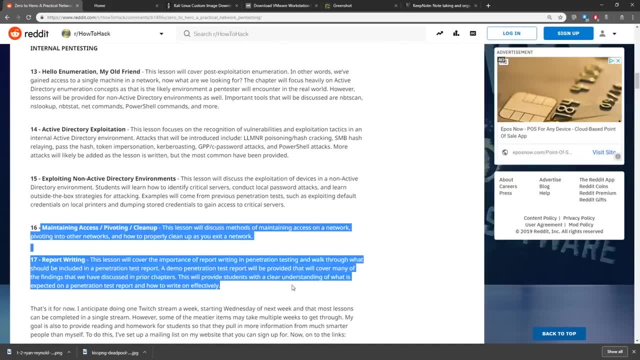 on actor directory. Um, we're going to focus on actor directory exploitation, non-actor directory exploitation. And finally, we'll talk about maintaining access, pivoting cleanup and report writing, And that's where we'll probably throw in that whole legal side of the house as well in terms 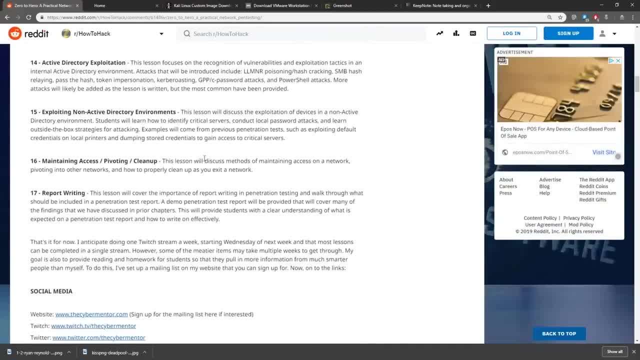 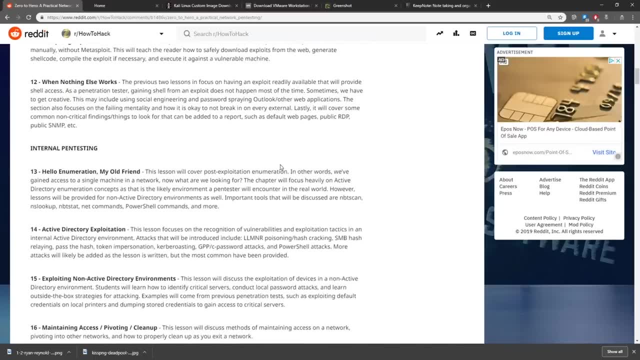 of documents. Um, so this is going to go week by week. If it takes longer than A week to do a lesson, it takes longer to do a week for a lesson, So I have no idea how long these are going to take. 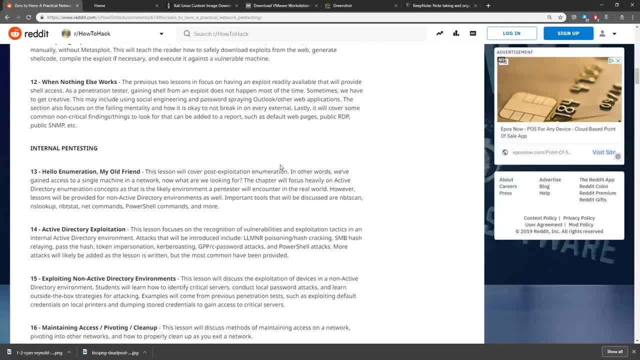 It's going to kind of go at our speed and where I feel that we're comfortable and I'm comfortable giving you guys- um, giving you guys advice, right? So I don't want to like skimp because I'm limiting you guys to one week. 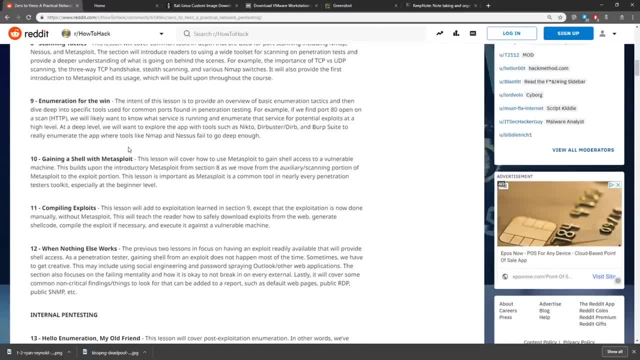 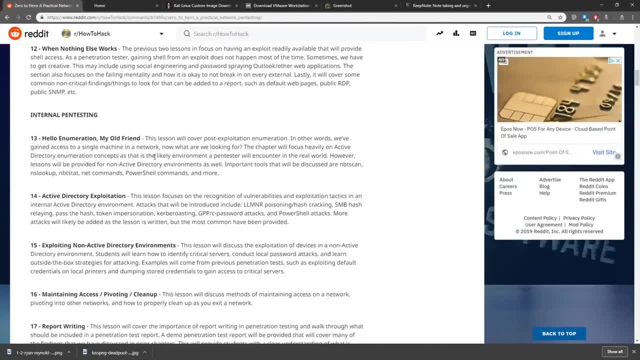 So I think that when it gets to some of the meteor sections, it's definitely going to take a couple of weeks and we'll get through it as we go. Um so, and in terms of that, we're going to be doing some setup lab environments. 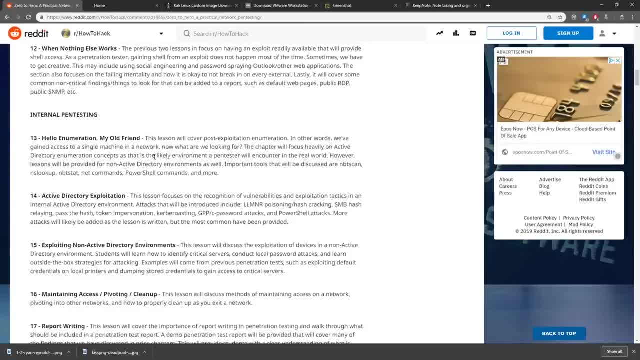 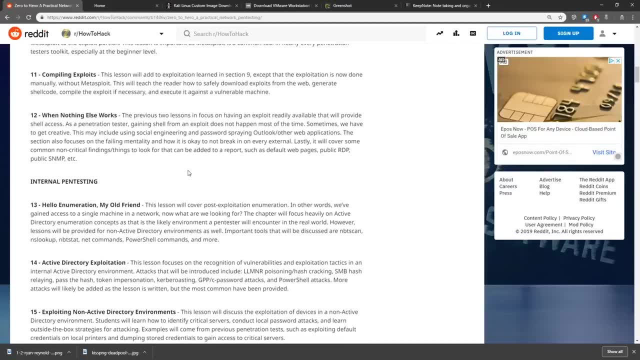 I'm going to do the best I can Get us what we can use. So Windows licensing requires payment. Typically, if you have a edu account, you might be able to get a Windows license for a server for. So there is some parts that you may have to watch and maybe not participate. 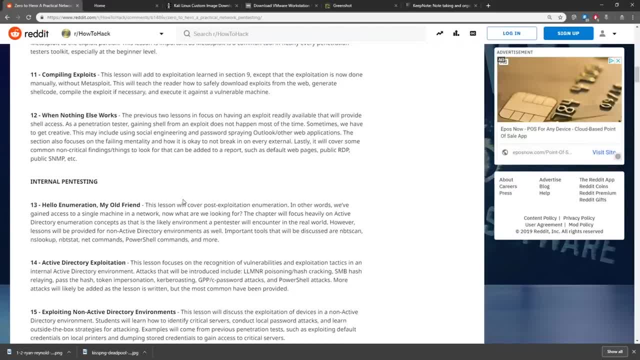 I'm working on that right now, So by the time we get to that, maybe that'll change. But the goal is to be able to build out our own server, make it vulnerable, exploit it and then learn how to patch it. 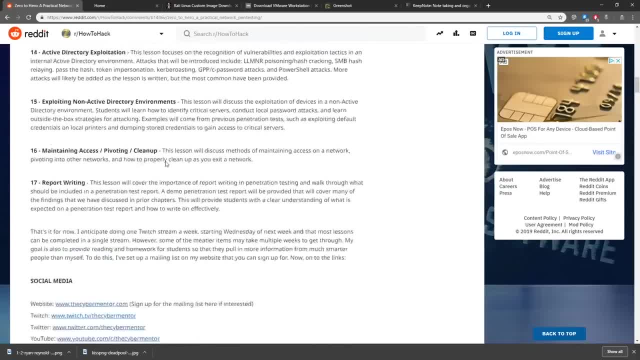 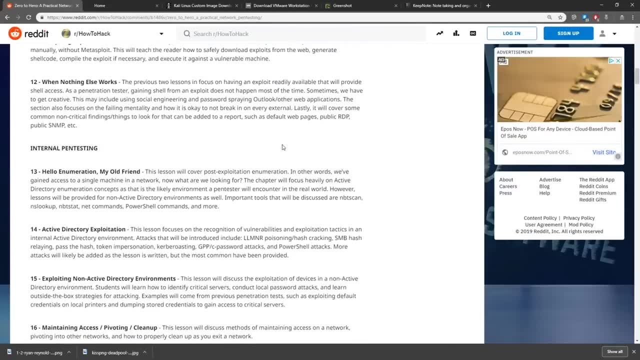 So we learned the red side and the blue side of the house. Um, so that's really it at a high level overview. I don't have all of these thought out into lesson plans. That's kind of going to be as I go. but most of these I have a general basic idea of what 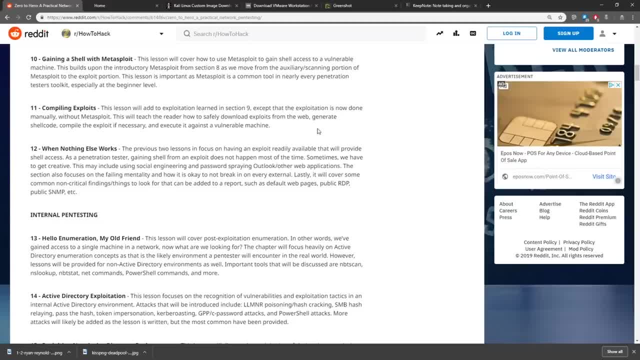 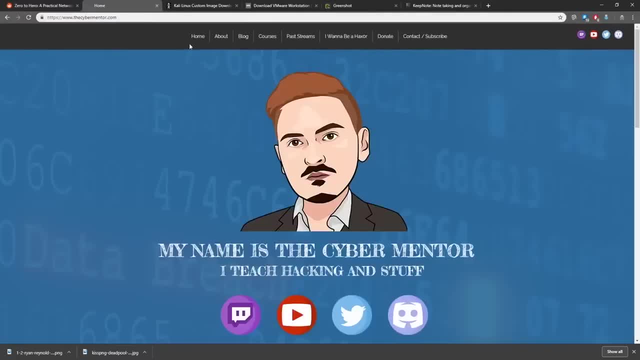 I want to do So. we're going to also talk about the important social links that I have. So if you come here, so if you go to the cybermentorcom- um, yeah, I was downloading some Deadpool stuff. You saw the Deadpool in the- uh, the live scene earlier. 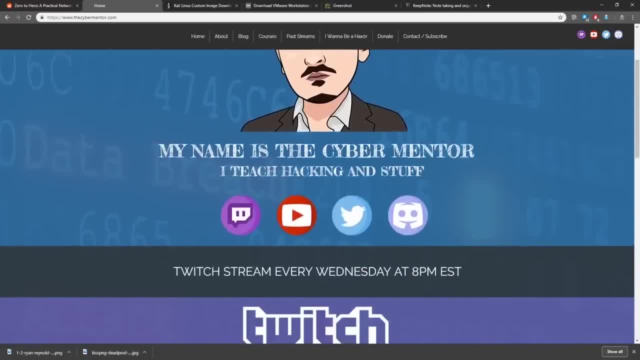 So what we're doing here with the- uh, the website is, If you have any of the important links you want to get to, they're all right here. So the Twitch. I have a YouTube channel as well, Like I said, where everything's going to be stored. um, in terms of VOD, I've got a Twitter. 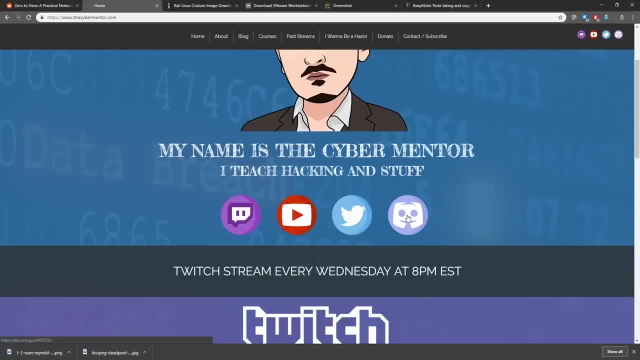 channel If you want to reach out to me, and I've got a discord channel, which many of you are already in. So, um, if you want to come chat with me or chat with other people that are like-minded, you're more than welcome to join the discord channel. uh, has a little bit of information. 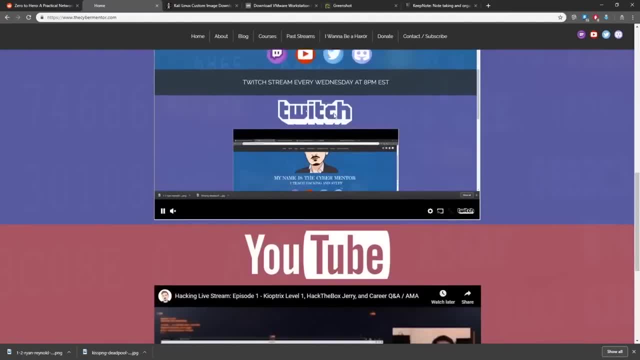 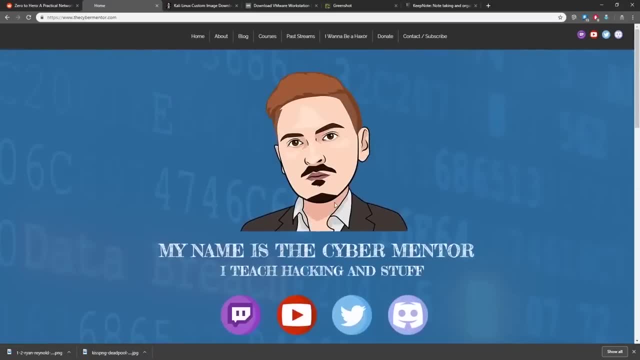 on the Twitch, You can see the Twitch is live, So we're kind of in a Twitch-ception right here. And then, uh, we've got the YouTube channel as well. Just a demo video, Um, so I am going to put it up in courses here. 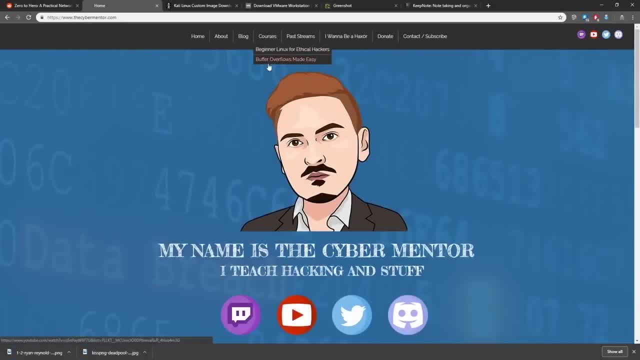 Eventually, I'm going to get it in where I have the information on the course. bring it off the Reddit site and put it into here, And then there'll be the VOD on the site as well. Um, you can also go to contact and subscribe up here. 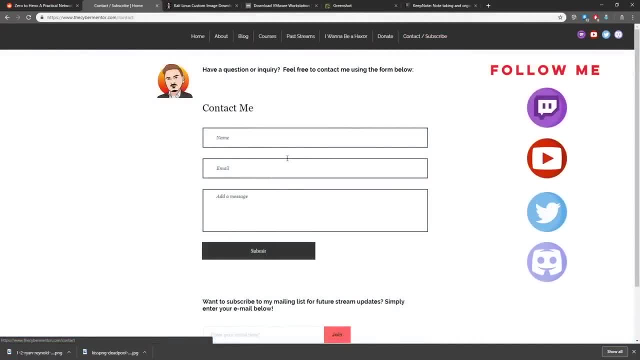 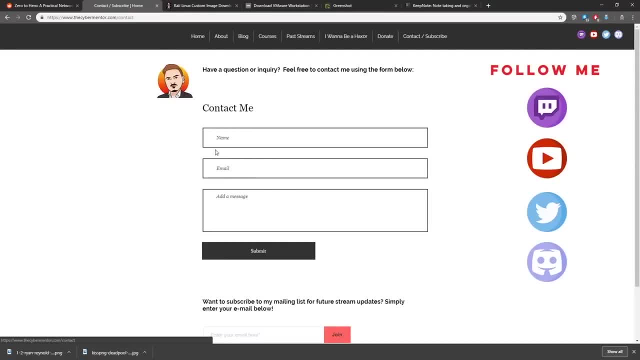 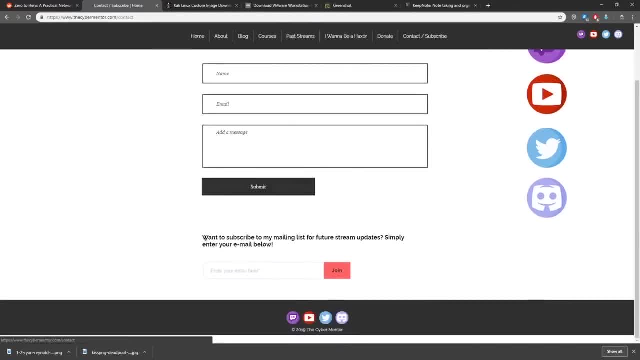 I'm way more responsive on those platforms. Um, and then for subscribing to the mailing list. then you come into here and you just say: put your email address and hit join And then what I'll do is on like the Monday or Tuesday before I'll send out any information. 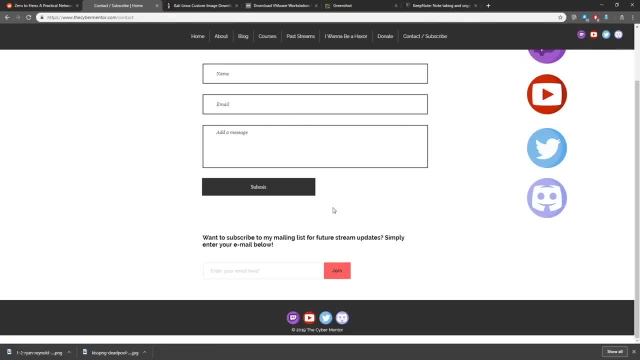 that you're going to need for that week. Um, for, for some lessons, like if we're talking about, like the Python lesson that's going to be starting next week, I may send you guys some things tomorrow to go ahead and get started. uh, because I 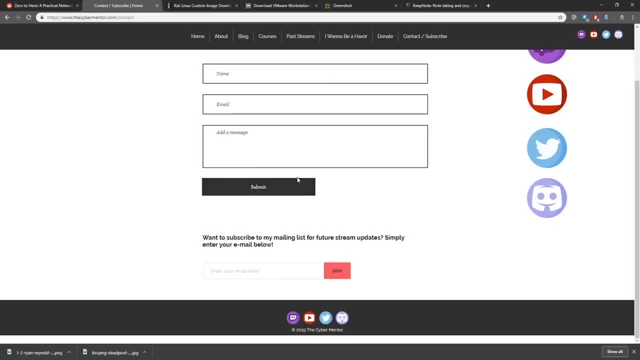 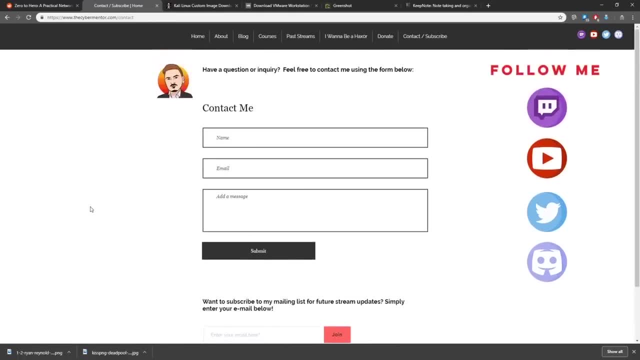 think I want you to have some information prior, like way, prior to the opportunity, prior to to study Python, before I even teach it to you. So anyway, yeah, I had a kissy Deadpool and a heart Deadpool, and I had to pick one because 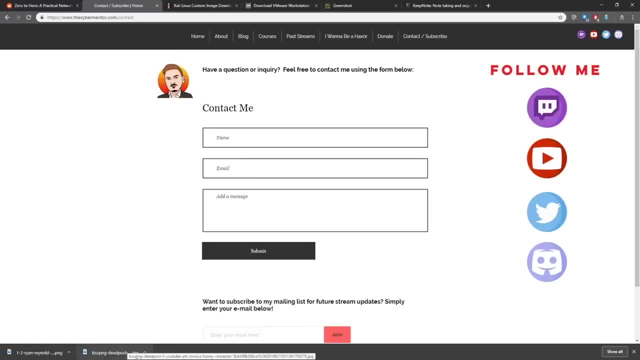 the one was a fake, uh, a fake PNG. It looked like a PNG but it ended up being a JPEG and I couldn't use the JPEG. So sad feels, bad man. Uh, so let's go back into the PowerPoint. 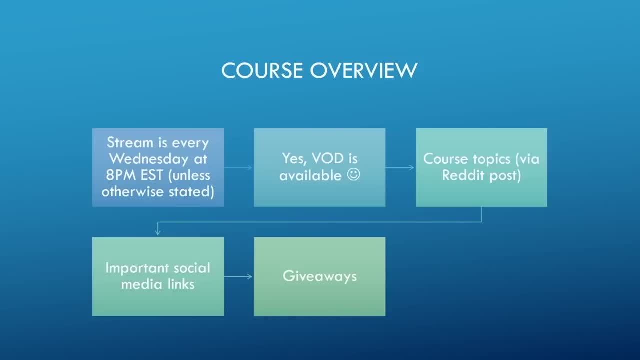 Let's see what else I've got for you. Yes, Giveaways, So I am going to be doing some giveaways. This is my personal stuff, So it's I would call lightly used or never used, bought and wanted, didn't really need. 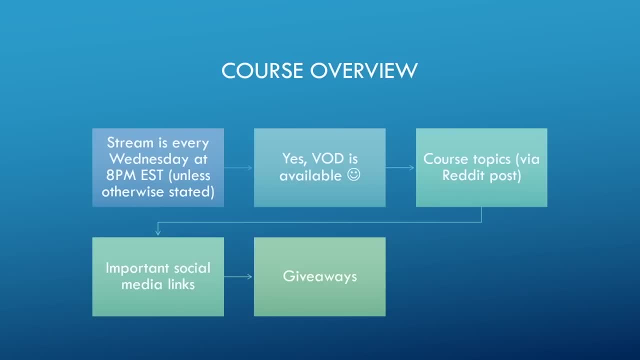 it or want it, um, or have a use for it. But some of you may have a use for it. Mostly going to be hack five stuff, um, like land turtle or a pineapple or packet squirrel et cetera. Got a bunch of random stuff. 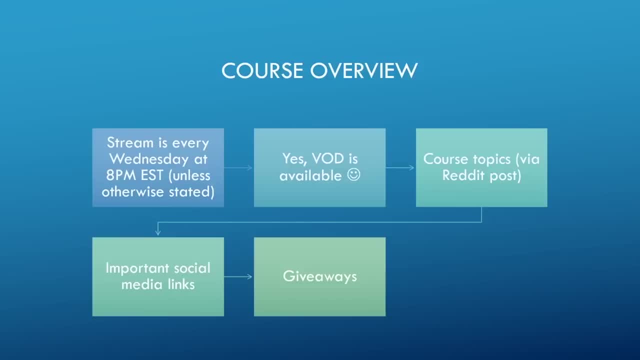 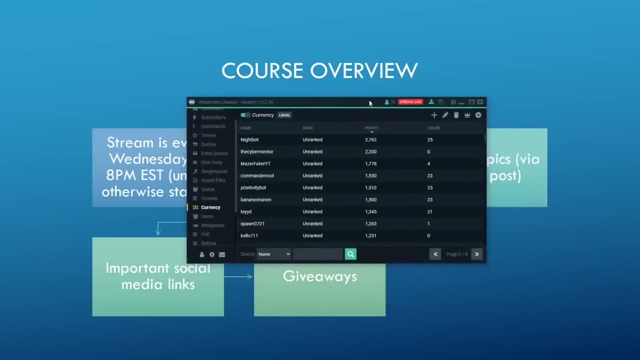 I really want to give away. Okay, So I'm going to share with you the how the giveaway works, So let me bring this over. So we've got currency over here. Um, so you could see by points: we've got the currency in terms of how much points you have. 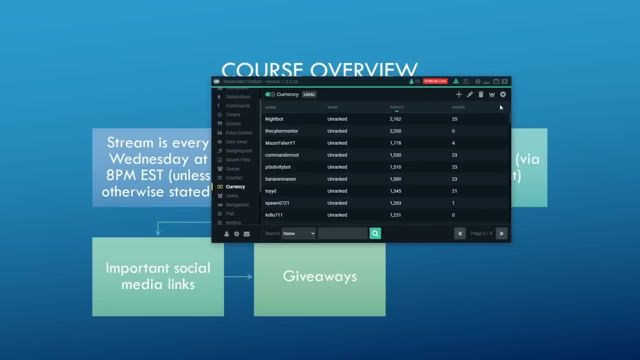 Right And basically the way I've done this is that you get points just for watching Um. so those who attend, those who show up um they they gain more points, and the points are how we're going to be um determining what we're. 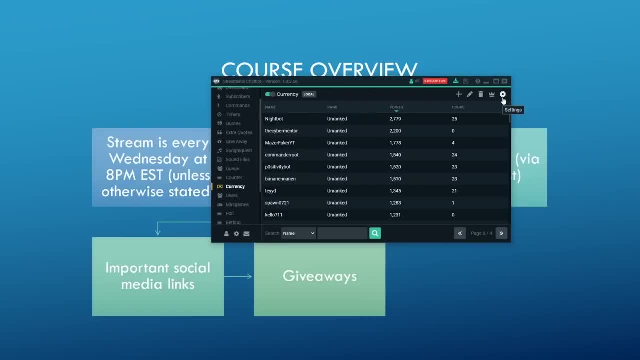 What we're doing with the giveaway. It's basically going to be a raffle, but the more points you have, the better off. you are Right, Um, so some of the settings that I have: you become a regular at 2000 points and we have live payouts. 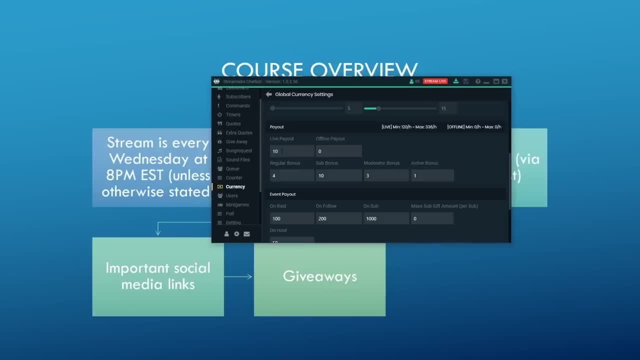 So if you're here, you get 10 points every- I don't know- 10 minutes or something like that. Or every six minutes- I don't know what. the rate is Three minutes, Um, if you're a sub, you get an actual additional 10 points. 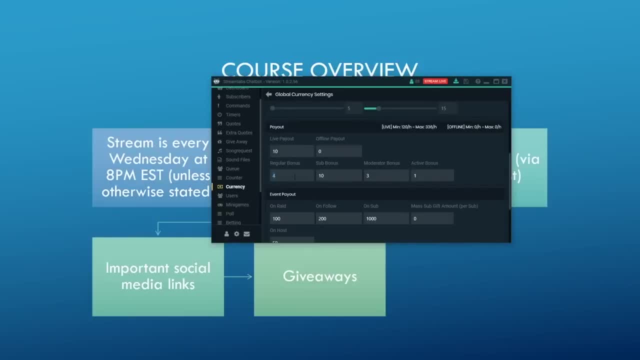 If you're a regular, like we just showed up here, you get an additional four points. Okay, Um. and then there's active bonus, which is an additional one point If you're on an event, which we are, So if you follow, you get a free 200 points. 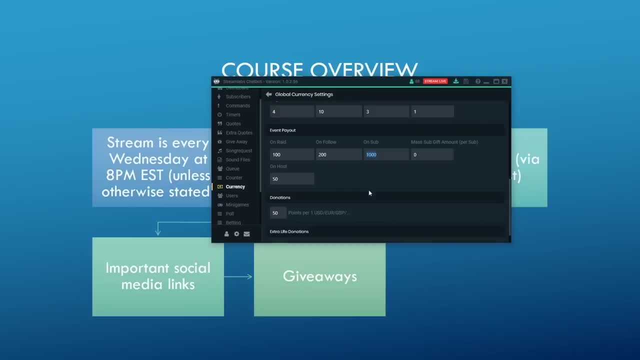 If you're a sub, you get a free 1000 points, et cetera. So this is just point systems, Um, and then if we come into, if you come into- mini games, there's some mini games that you guys can play. 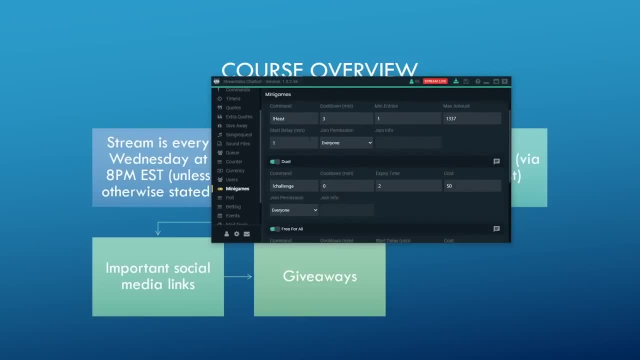 If you're bored or whatever, you guys can play these little heists or duels or whatever you want. You risk points, So win uh, win currency or whatever. So it's gambling for those who who want to gamble. Uh, they are on a time delay and a cool down. 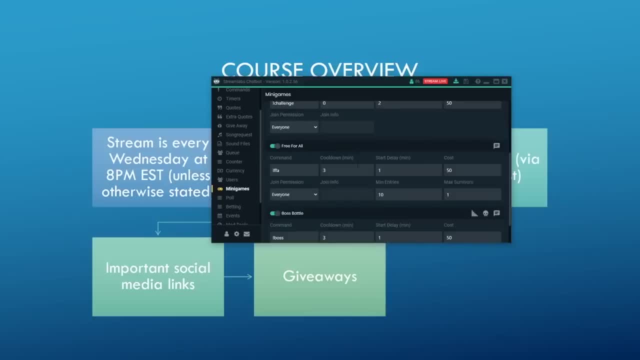 So, like the heist that you just ran, uh, you're trying to get a heist together. Everybody who types in heists at a certain point will get into that heist within X amount of time. Um, and then it just kind of goes from there. 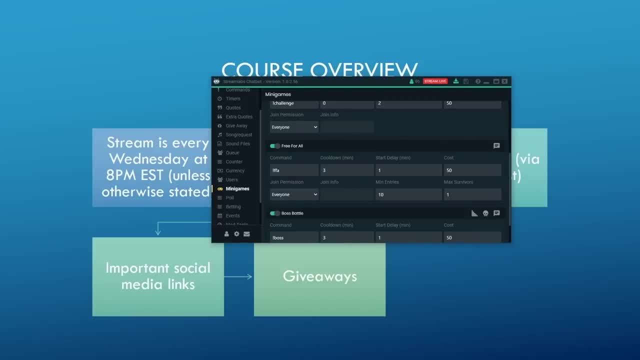 And thank you so much. Everybody who's subscribing right now. Um, thank you. I should say thank you. Sorry, Snatch hammer bammers. Uh, let's see, Go down The list. uh, chloro shoe. 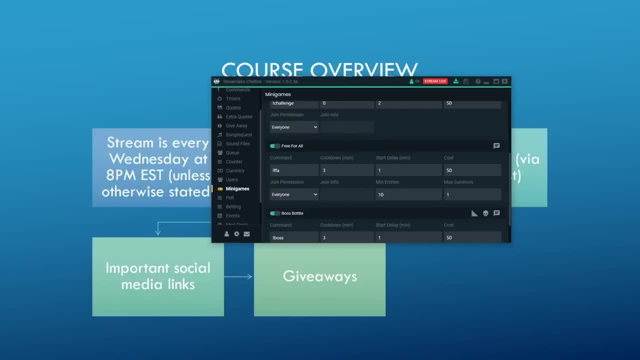 I hope I said that right. Riveting bug: uh, POMF gaming, reckless pancake. Thank you, guys, everybody. Um, and so the last thing is: when we go into the giveaway, where is the giveaways? So if we go into giveaway, we're going to do a raffle for a prize. 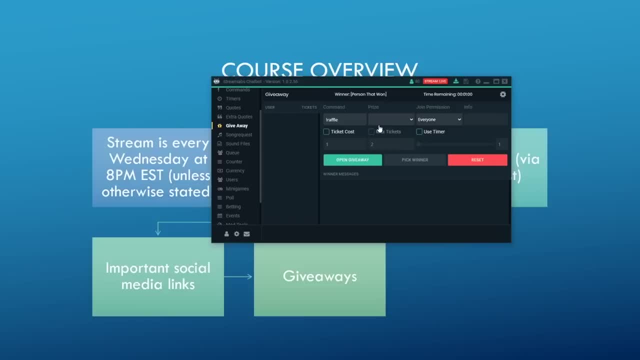 I haven't determined how much, um, I haven't determined how much it's going to be yet, but what we're going to do If you come into settings here I've given a little bit more luck to regulars and a little 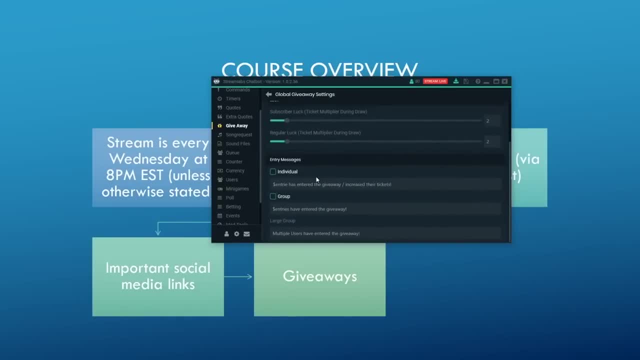 bit more luck to subscribers. So again, it plays in your favor to be a regular, to attend um and to watch these streams. So the students who come in here and they watch more frequently, you guys are gonna have a better chance of these giveaways. 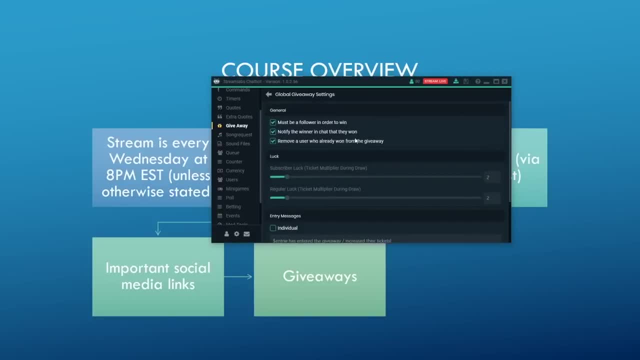 Um, so in terms of getting a discord, I have not yet for the subs, but I will do that. That's a great idea. So, yeah, it's rigged. You guys lost all your money. I'm sorry. This is what gambling is. 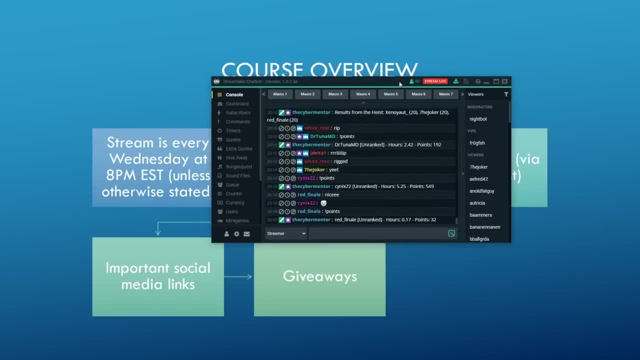 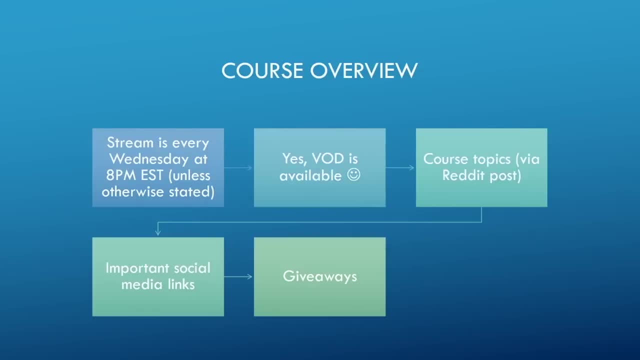 Gambling does. It's a lesson in life. So that's really it. So on a random night, any night uh that I stream, I may give something away. So if you guys are are watching and you uh are here for the giveaway, then you'll. 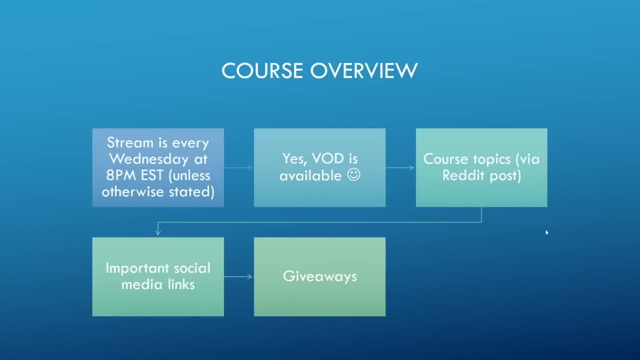 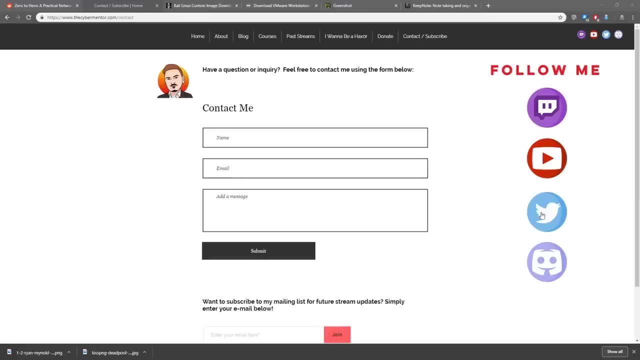 have the opportunity. Um, and thank you, Mr Deviant, for the sub. So that is that for the course overview. Let's go ahead and move on. So the first thing we're going to talk about is just really, really, really, really really. 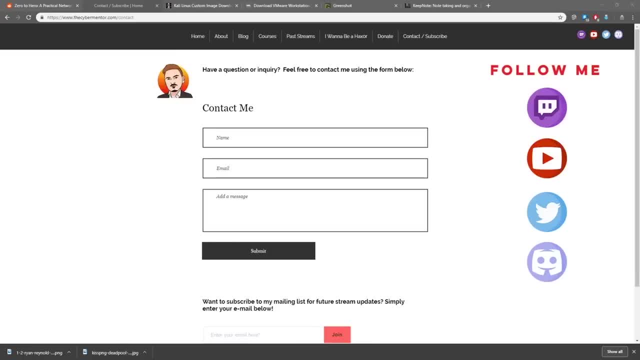 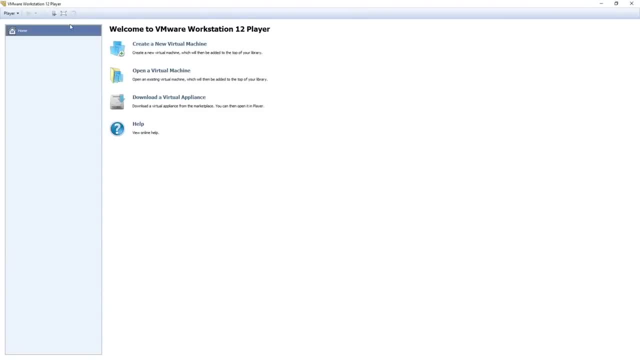 really quickly installing our Kali Linux, So you should by now have open your VMware workstation. I'm on 12 players still, So you're probably on like 15 or something. It should look very similar. The aspect of what we're going to do is we're going to go into player here. 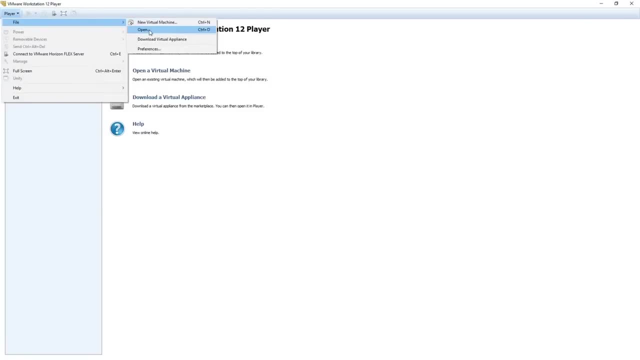 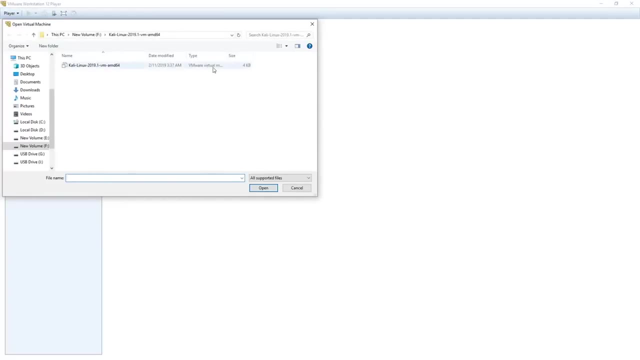 We're going to go into file and then we're just going to say open And it goes right to my folder here with this, this virtual machine, this VMware virtual machine, So this four kilobyte little file here. what we're going to be doing is we're going to 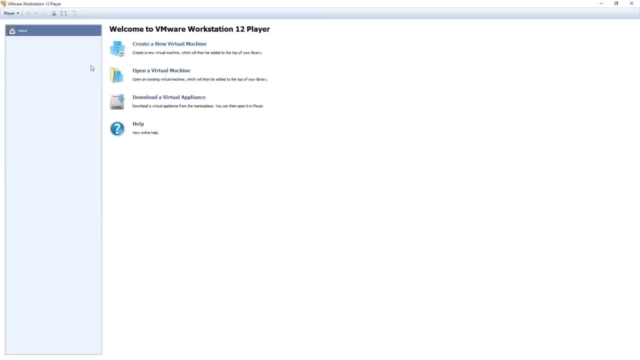 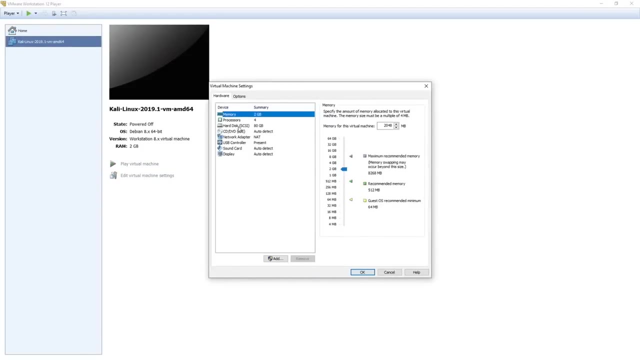 double click on it And then we got a couple of settings that we're going to add here. So what we're going to do is we're going to say, okay, how much memory do we want? Well, how much memory does your computer have? 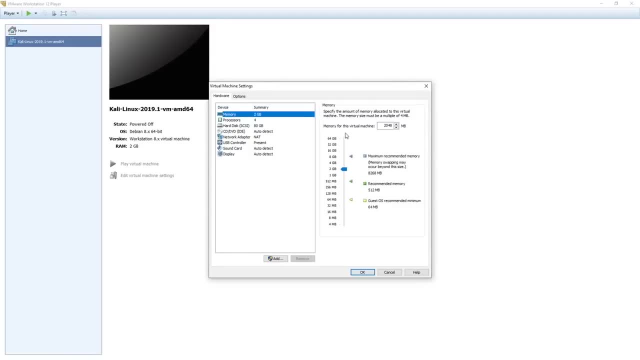 Like, the computer I'm running on has 32 gigabytes of Ram, So I can Jack this up a little bit If I want to. I typically put it at eight. If you're running on 16 or less, I would put it at eight. 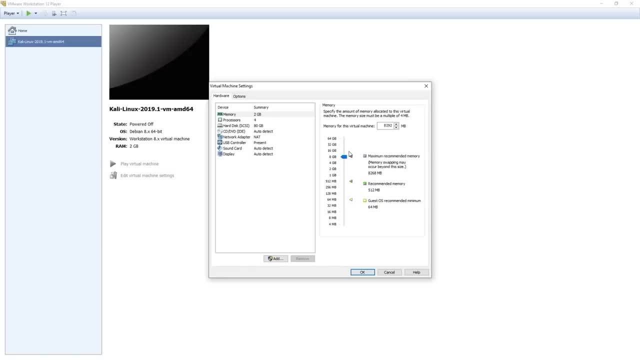 Okay If you're running on less. I would put it at four probably, But it's up to you. The less Ram you have, the slower it's going to go. Also, this creates like a page file or some sort of file that eats up this amount of space on your hard drive as well. 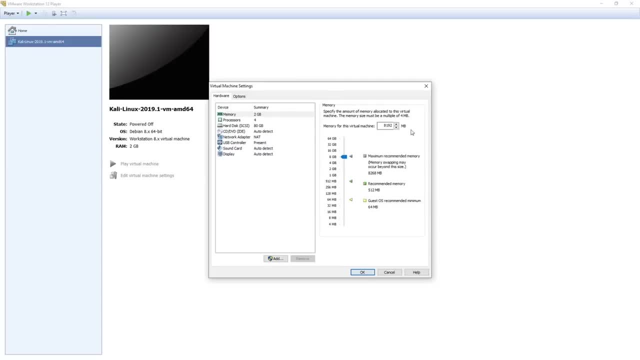 So expect eight gigs of space to be eaten up on your hard drive. So if you don't have a room, be very cautious of that. The other thing we need to set here is your network adapter, and we need to make sure that that's set to NAT and not bridged. 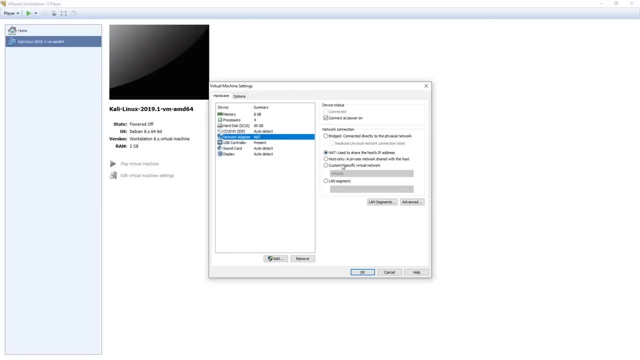 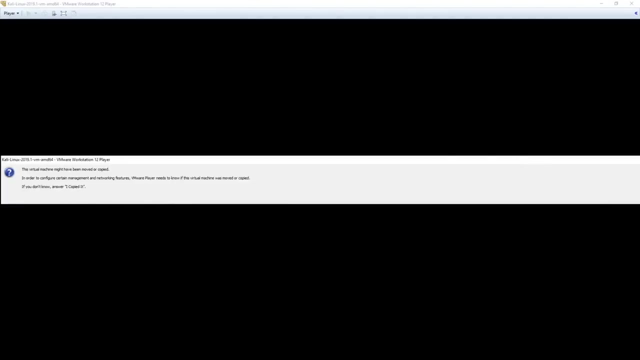 So we'll use NAT the whole course And we're going to say, use the share, the host IP address, That's fine, Okay. And then all we're going to do is hit play. And that is asking in the weirdest thing I've ever seen. 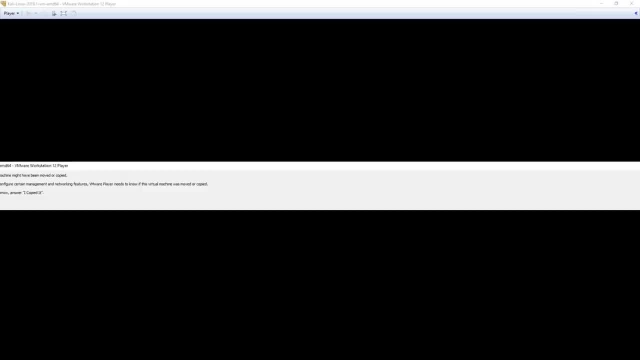 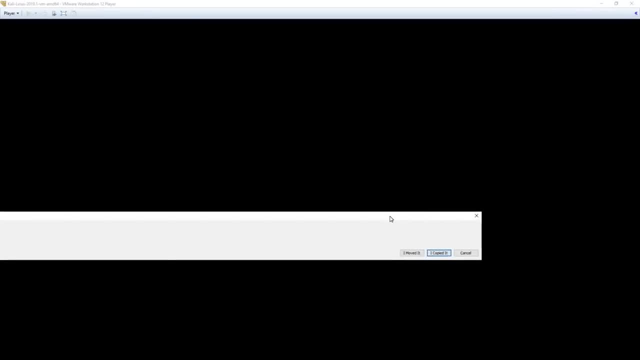 This is like a two foot long. I don't even know how to describe. Look how long this is. I've never seen this before. Anyway, it's going to ask you if you see in here it says I moved it, I copied it, or cancel. 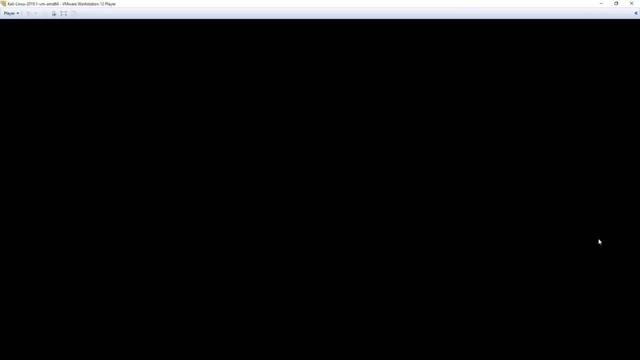 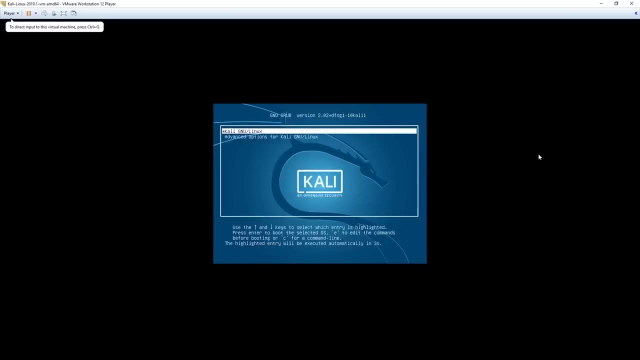 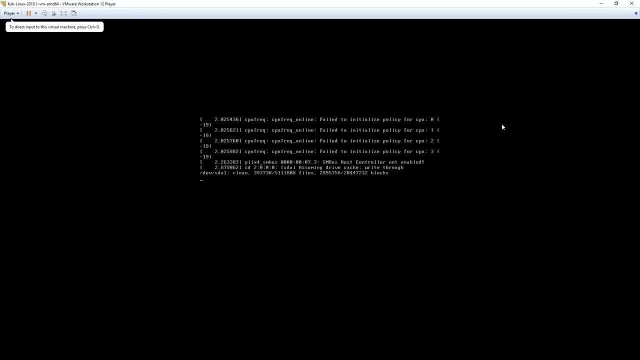 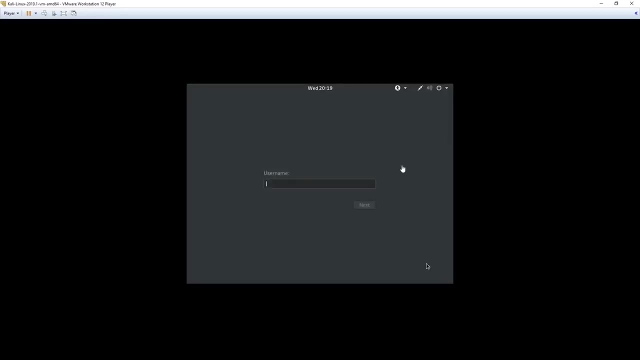 You're going to say I copied it And it should boot up. Yeah, I copied that, mofo. I've had more stability with NAT over bridged. I know some people like to run bridge and I used to run bridge, but I've always ran NAT. 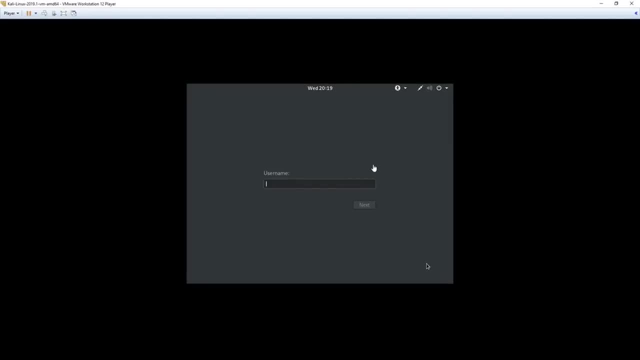 The only time I run bridge is when I'm doing an external assessment or something where I'm not using it, Or something where I want to have a dedicated IP or whatever. Like I can do port forwarding specifically to the IP address, if that makes sense. 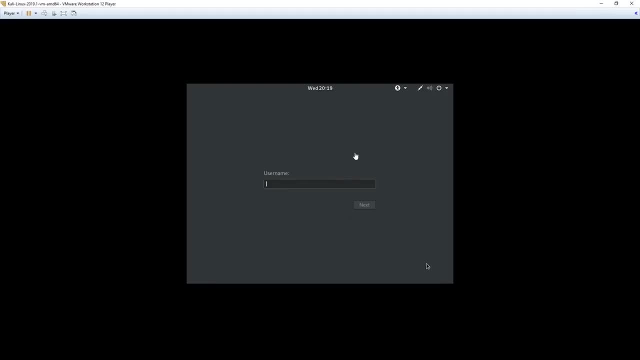 My router is incredibly weird, So I have to have bridge connection for that. But other than that, I like using NAT. You guys can do whatever you want, But if it doesn't work because you use bridged, don't yell at me. 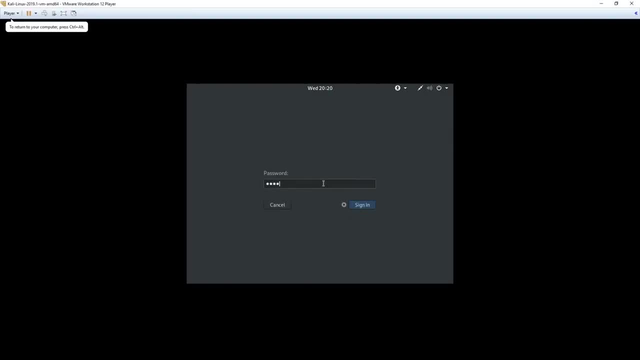 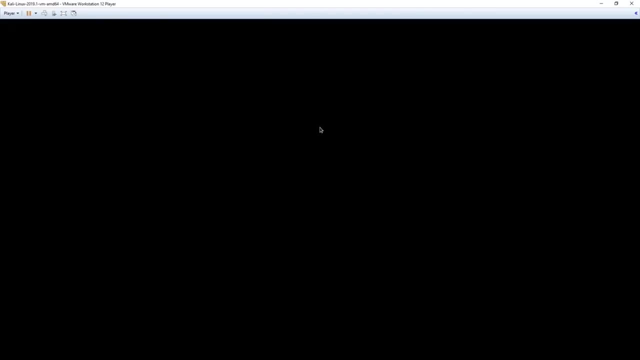 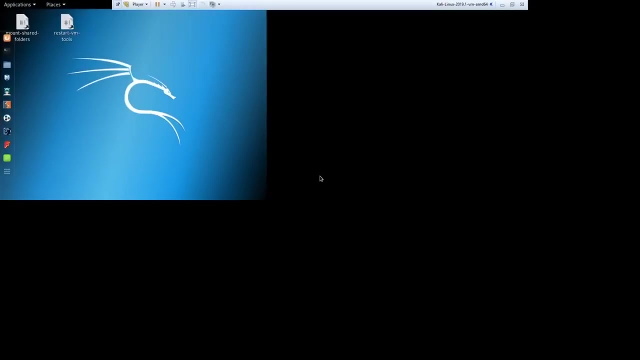 So username is root, Password is root, backwards T-O-O-R, And that will get you logged in to your machine. Well, Kali, you're special. All right, so here we are. This is our Kali Linux machine. 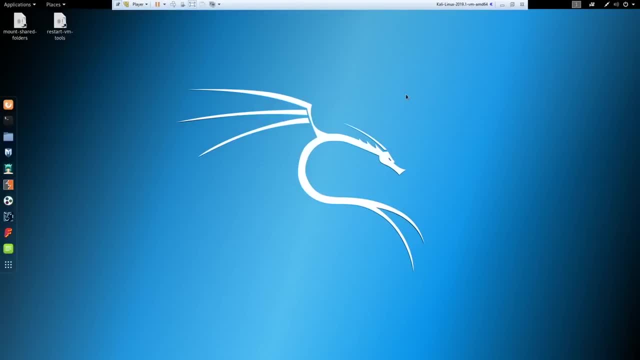 This is our distribution of Linux that is made for pen testing. So when we come into here, we have some things on the side panel. here our favorites. We'll talk about some of these tools later. You'll definitely be using some of these. 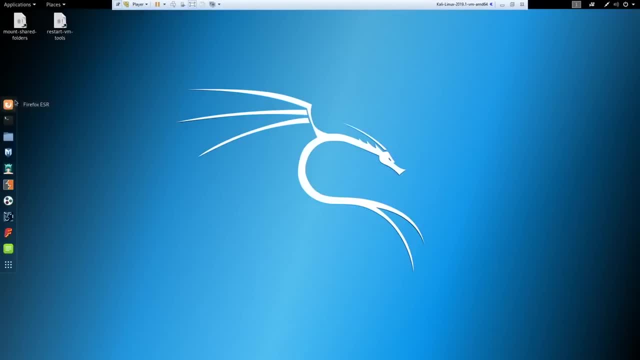 Most important ones to know is this little ice weasel. here is your Firefox. I guess it's Firefox now, And then your terminal is right here. This is where we're going to be living most of the time, So the first things first. we're going to have our first minimal lesson here in Linux. 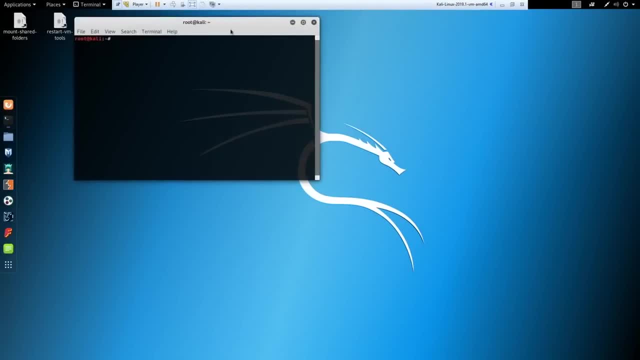 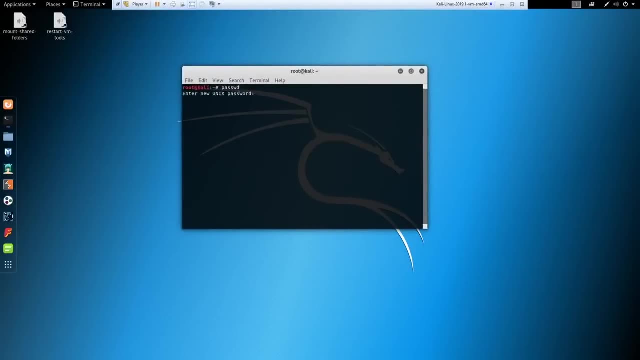 I want you to click on this terminal and open it, And then we're going to change our password. So we're just going to say P-A-S-S-W-D And we're going to enter a new password, because we don't want to use the default password. 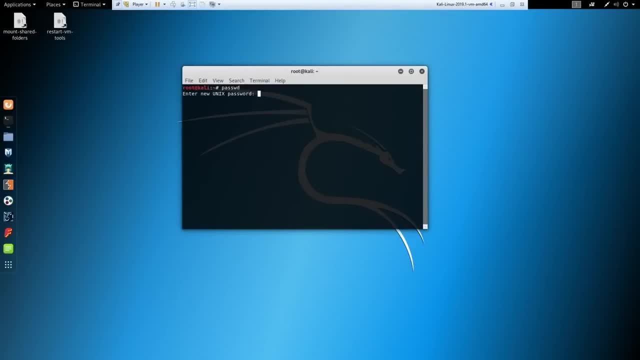 So what we're going to do is we're going to go to our terminal, So what we're going to be doing here is whatever you want it to be, and then do it twice. All right, So now we've got our password set and we are good to go. 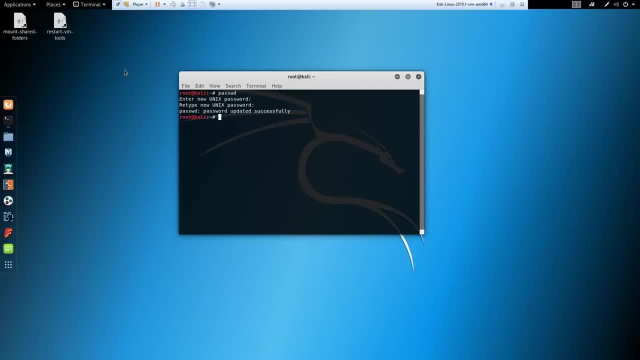 So we're going to put a little back burner on Kali for now. We're going to cover Kali in a little bit more depth here in a few minutes. We're actually really doing really well on schedule, So we'll have some more time for either Q&A or questions when it comes to the introductory Linux section. 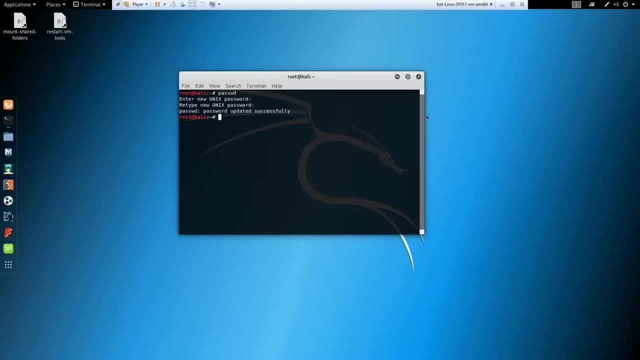 So when we do this, what we're going to do is we're going to go ahead and talk about note keeping first, Because you actually have a built-in note keeping application in here. So if we go into, I don't even know where it is. 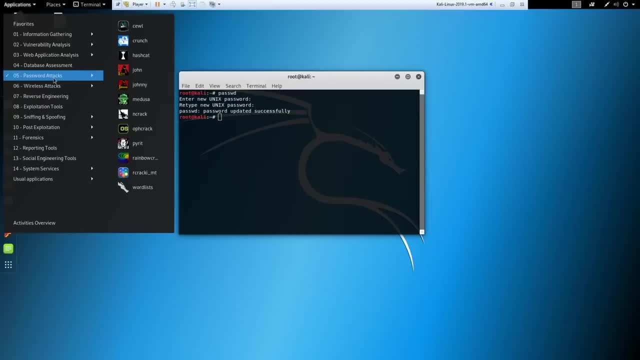 Definitely somewhere in here. You guys know where it's at Useful applications, maybe Evernote. Yeah, let's use Evernote. There's Cherry Tree. Okay, So they took it out. actually, They have put it used to be keep note. that came with this. 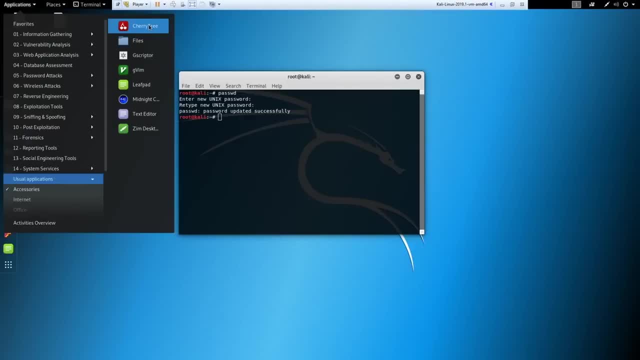 Now they've moved it to Cherry Tree. Oh, keep notes discontinued. That's sad. Well, you guys can use whatever you want. So if you want to use Cherry Tree, We can open up Cherry Tree And you can come in here and learn about this. 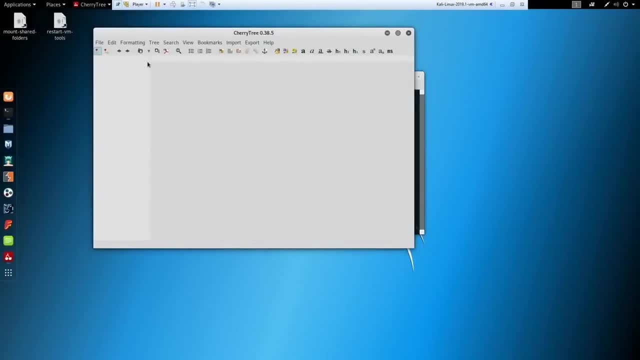 For this lesson, in this course specifically, I'm going to show you what I do with keep note And we're going to go from there. But I don't like actually keeping my notes inside of my Linux machine. I like keeping my notes on my Windows machine or whatever you're running your VM from. 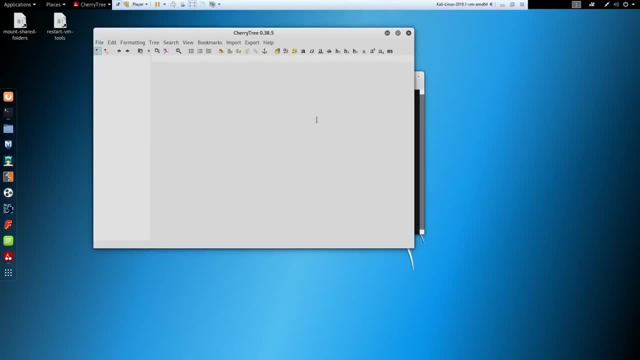 Only because if, for some reason, your machine crashed or you didn't have a backup or whatever, You lose all your notes. You lose everything, So definitely worth keeping them external. The only reason I want to show keep note is because I thought it was in Kali until just now. 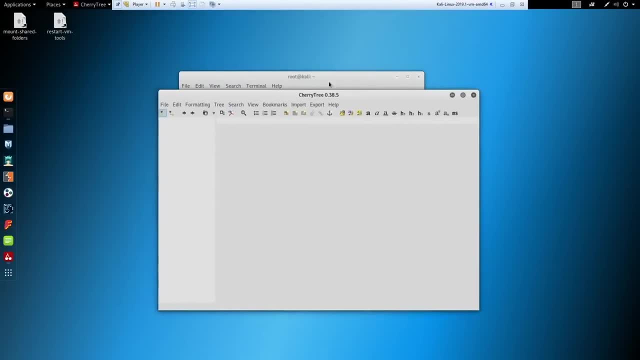 So joke's on me for not knowing that, But Cherry Tree is a very good alternative. I know some people also use Atom as well, Depending on if it works for you or not. But let me go ahead and bring over my keep note. 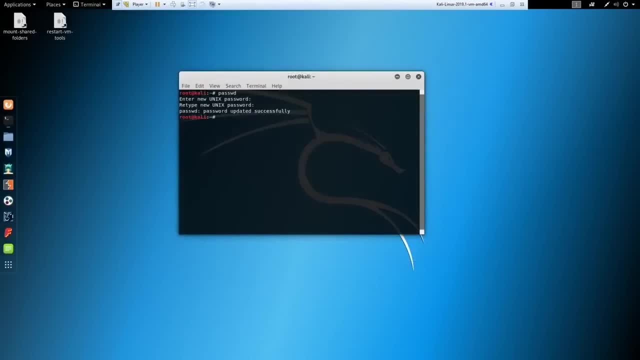 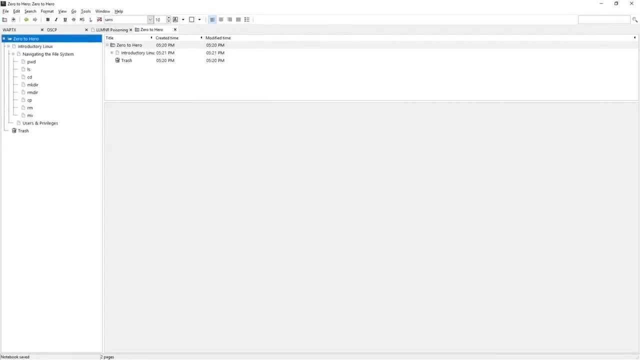 And I'm going to show you some examples of how I take notes. So when we're here and we're looking at the notes, I'm starting here with the zero to hero and how I kind of like to take notes. So if we're doing introductory Linux, I'm going to break this down kind of into sections tonight. 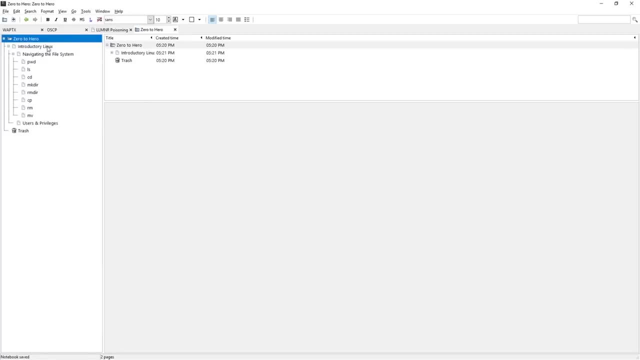 And what we can do is: okay, say, I want to do introductory Linux And I'm going to be covering something called navigating the file systems- How you get around the file system in terminal. If we look through here, there's a bunch of different commands that we're going to be covering. 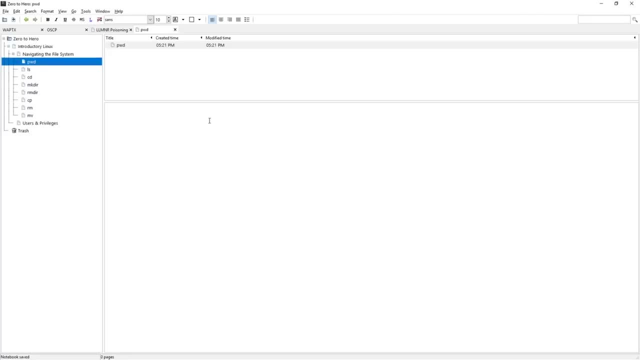 And we can go into here and like click on them And we'll have notes for each command. That's one way of doing this. So you kind of have topic subtopic and then sub-subtopic, Very, very organized, And another way to do that is: okay, I don't want to have all these little sub. 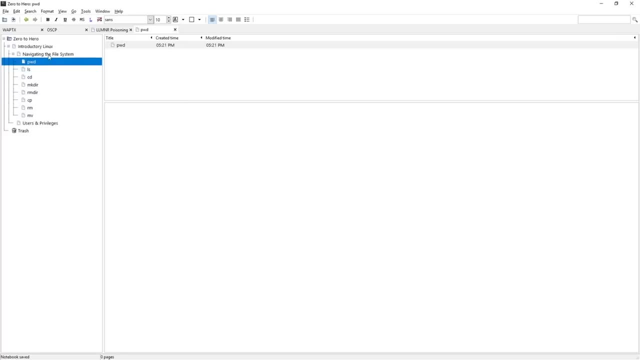 They're called children or child categories. Instead, you can just come in and put them in here, So you could say: print working directory- Okay, Here's a picture of what that might look like. Or change directory. Here's what that might look like. 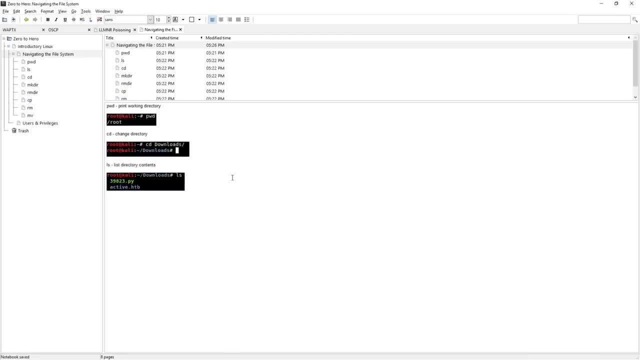 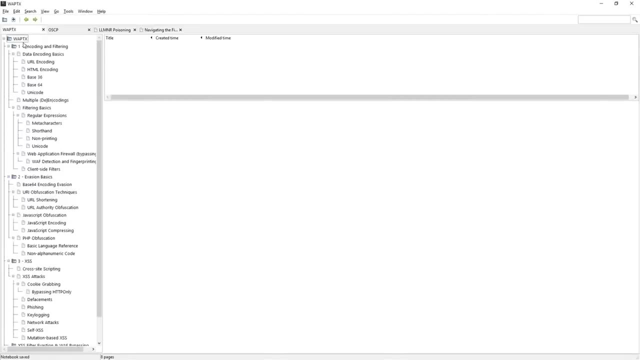 So you kind of just go through. Now, when it actually comes down to things, I'm going to show you my notebooks, So without clicking on anything because it is confidential information. So I'm taking a course right now, WAPTX through eLearn Security. 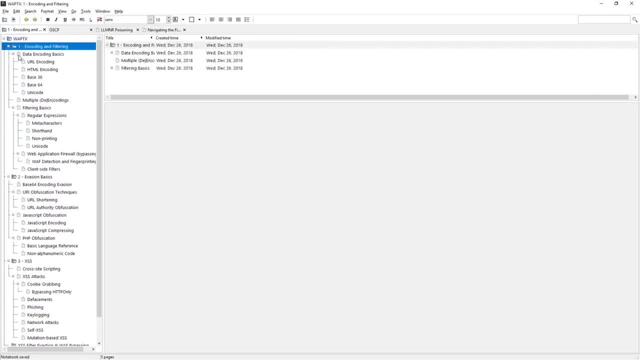 You can see that I actually create a folder for the chapter And then they have subcategories, Right, And then they have lessons inside of those categories. So for data encoding basics, I have something for URL HTML: base 36,, base 64,, et cetera. 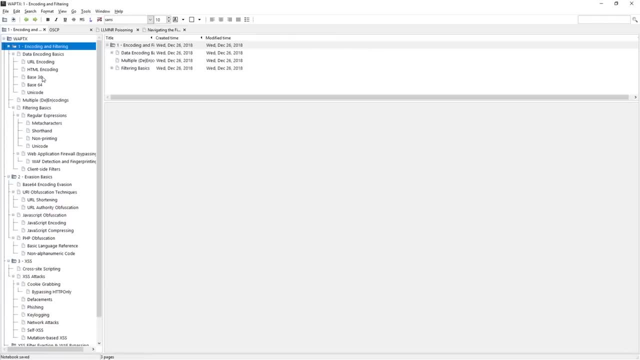 I break it down to the very specifics because if I want to search through this and I want to know something right away, I can kind of just come down and drill down into these and find it really easy. We're not looking through any sensitive information. 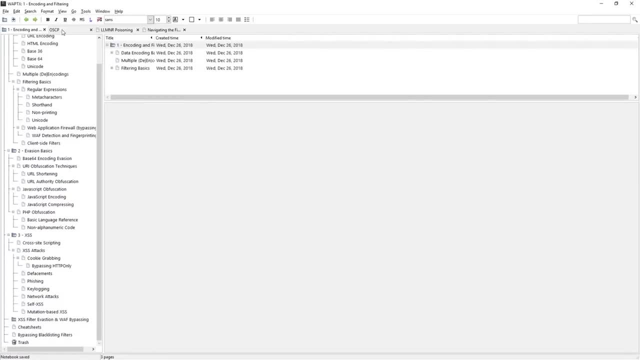 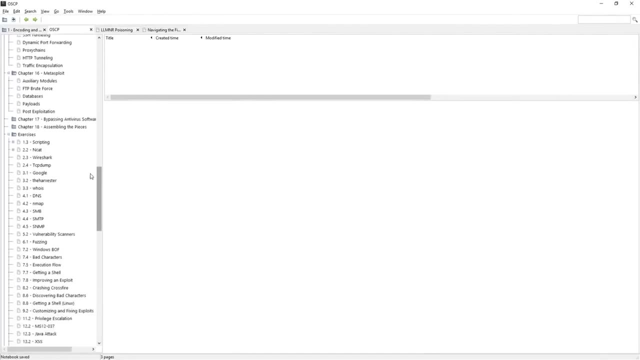 This is all in a syllabus, my friend. So OSCP, same thing, Like. look at the notes, The amount of notes that I took during the OSCP And they're all done by chapter exercises and machines, Right. 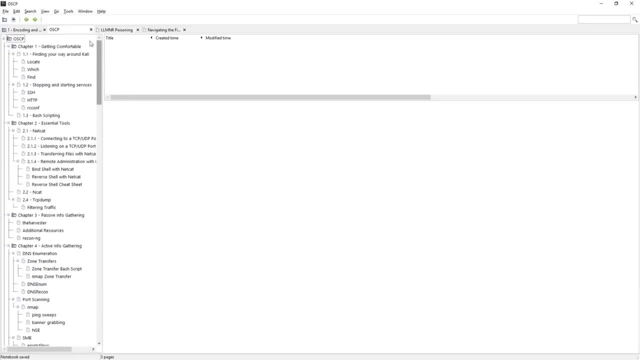 And that's without showing you anything at all. Right, You're going to see the amount of data that I put in here. So again, you can see chapter 1,, 1.1,, 1.2, and even the subcategories as well. 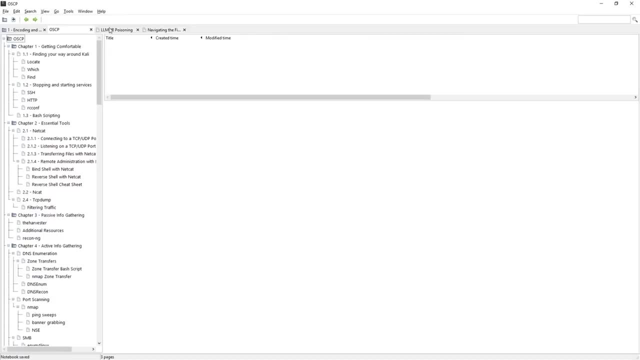 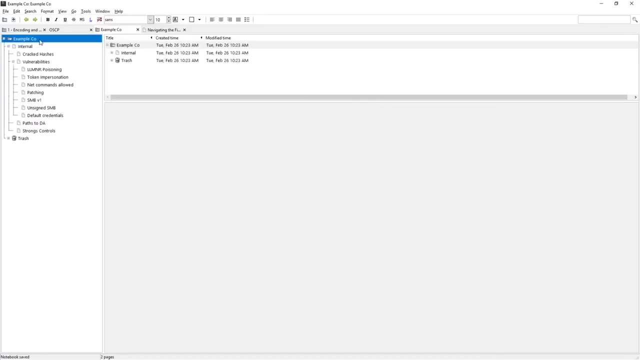 So when we talk about a real client, sometimes if we're going through a real client and this is kind of an example company, I've kind of blurred it out. I've kind of blurred it out because I had to take pictures and just show you. 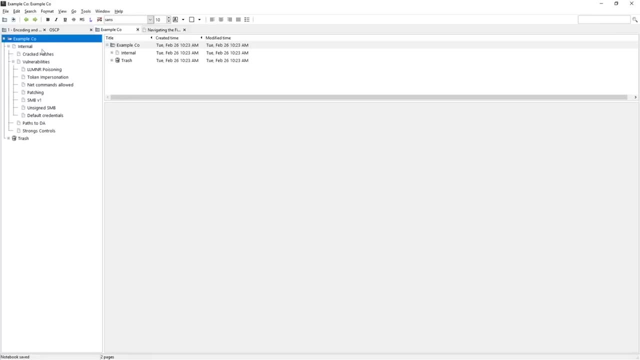 So I made this example company. This was an internal assessment that we did. And you come through here and say, okay, well, I did an internal assessment. What are some things that I have? Well, I have cracked hashes that I found. 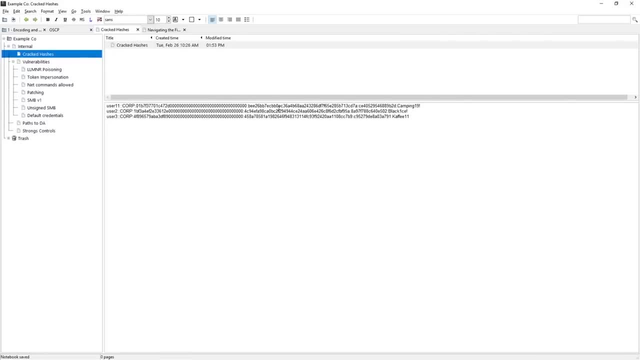 So if I have some cracked hashes for user 1,, 2, 3 at corp, These are the hashes, the passwords that I found. I might be able to use those later. Just some notes for myself: The vulnerabilities that I find. 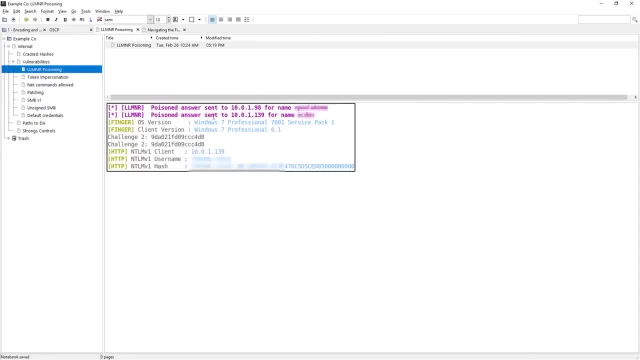 So if I come in here and I say, okay, well, I found LLMNR. I found LLMNR poisoning, Here are the usernames, the hash, et cetera, the machine that I found it on, whatever, This is just a proof picture. 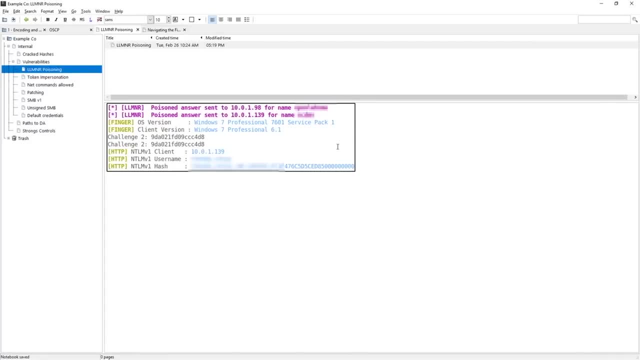 And I'll show you guys how I'm taking screenshots. We're actually going to get to that. So when you come through here- same thing token impersonation- I come through and I say, okay, here's the screenshots that I do. 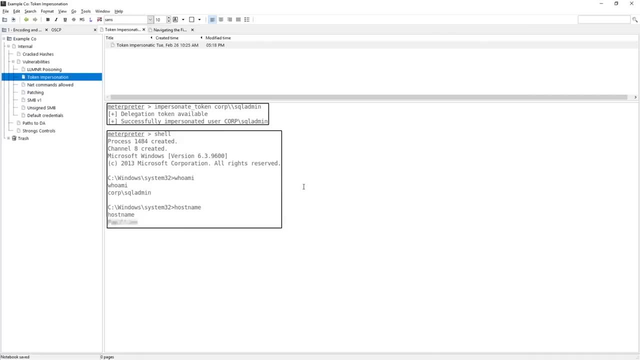 And what you want is you want as much information as possible. Now, this here, what you're looking at, It's actually me doing a rush job. I am not in here like on any of these. You don't see me putting in for a lot of them, like the machine I was on, what time it was at. 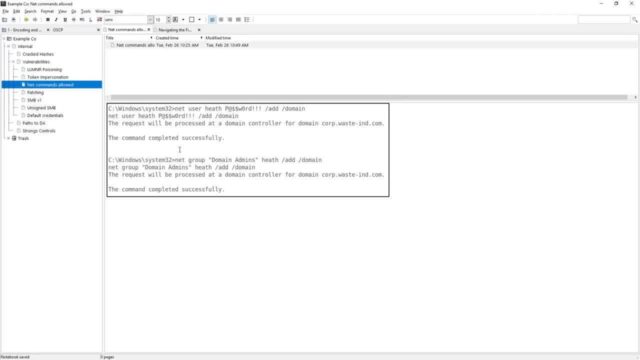 You know as much information and detail as you can get possible, the better. What I do with these is when I go back and I sit down and I write my report. I come in here and I say, okay, well, there was LLMNR poisoning. 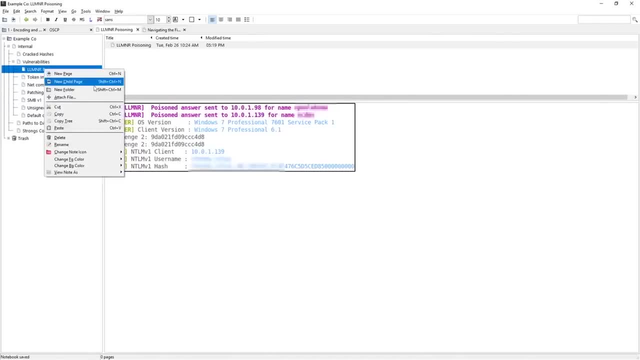 And then what I do is I say, okay, well, let me write that in. And then what I'll do is I'll say, okay, I've written that, So then I put a check mark next to it. I know I wrote it. 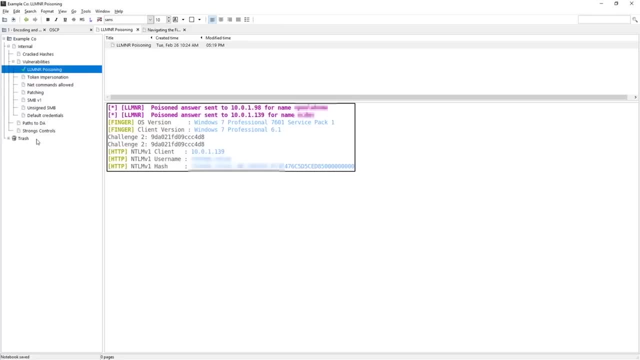 And then we come down here and we do that for all of them. And then some other things that you want to know is you say, okay, what paths to domain admin did I have? So for this one we did LLMNR poisoning. 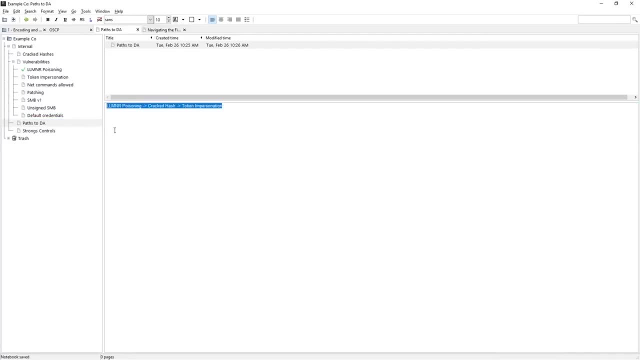 We cracked a hash and then we did token impersonation to get domain admin. What strong controls do they have? Well, they caught us scanning. They caught us when we created the domain admin account. Just some notes that you have in here. The more detailed the possible. 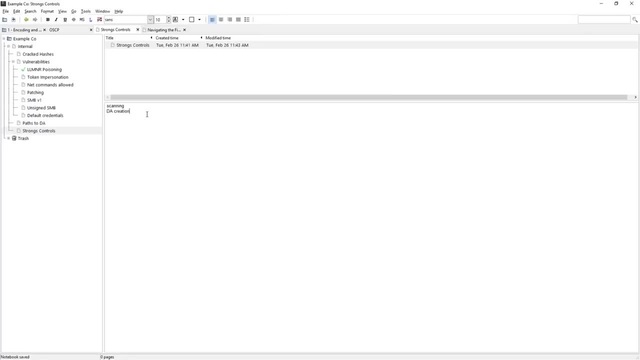 As you can see, there's not a lot of details in here. When you came in here, all I've got is the screenshots, not really a whole lot else. Now, many of you are asking what my screenshotting tool is, And I prefer GreenShot. 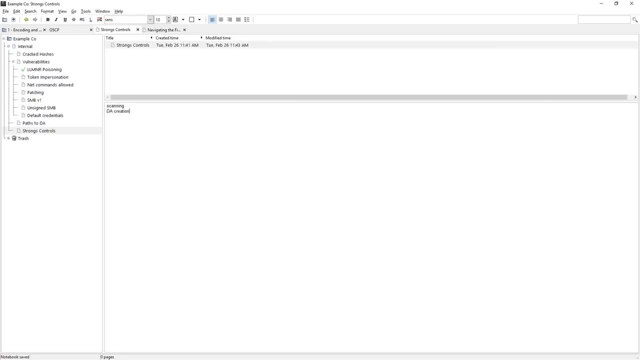 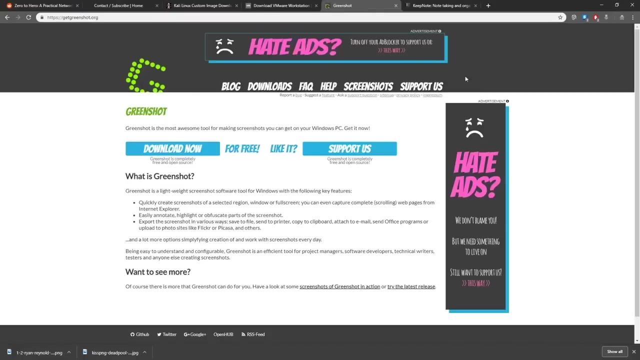 And I learned today from Kelly that you actually cannot use GreenShot on Linux, So you're on your own for a Linux solution. But if you come out here to GreenShot, it's very nice. All you have to do- for me is all I do- is hit print screen. 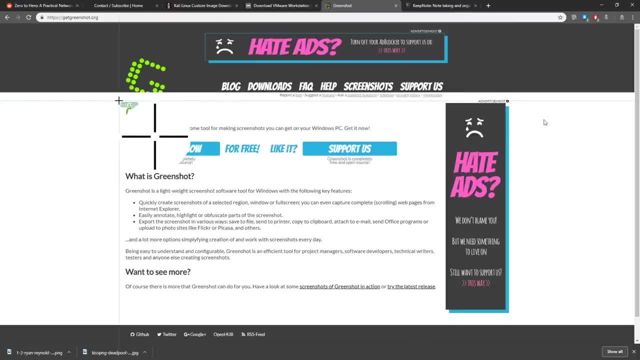 And if you guys can see this, you can't- But you basically get an arrow here and I grab it and I can just select the screen like that right, And then I can say: open an image editor here. Let me drag this over for you guys. 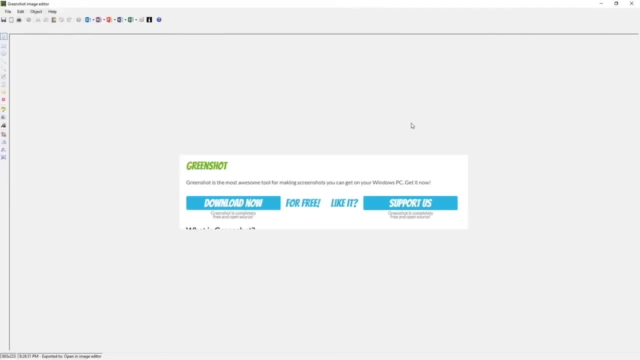 So I just took this little screenshot. It zooms in for you. Oh, you can see. it freezes my screen on my end, Sorry guys. And so some of the nice things that it has. like you come in here and you got effects. 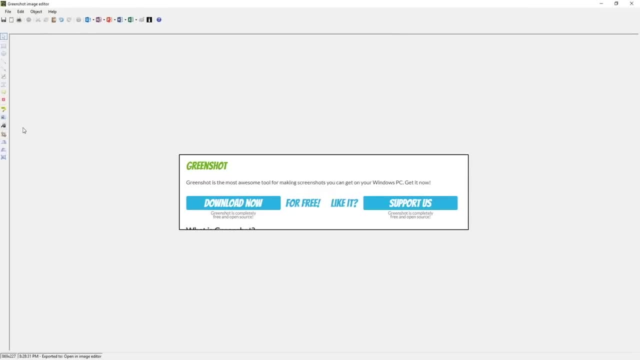 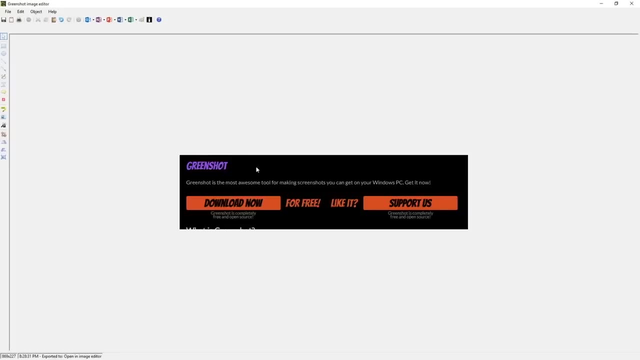 Like I like to put a border on my pictures. Okay, Automatic border. If I'm running like a black Cali, I can invert the picture and make it white. So, like for the reporting and stuff, you don't want a black screen. 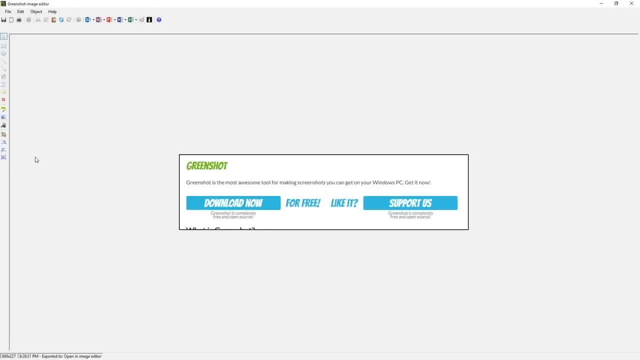 You actually kind of want white on the background. So if you're taking screenshots of the black background, very nice to have. It's got a highlighting tool. So like I want to point out something specifically on that screenshot. Really nice, It's got obfuscation. 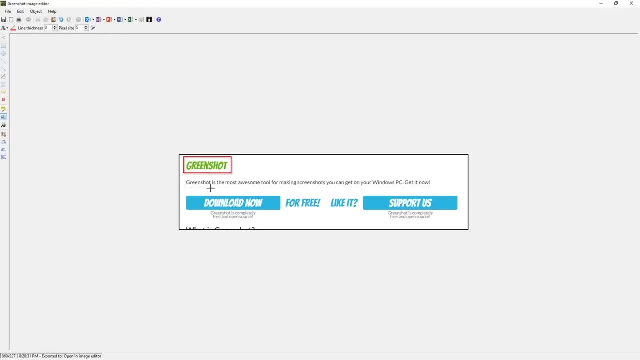 So if I wanted to blur out the image, I could do that. If I want this word here, I could just say: okay, I want to blur that word out. So this tool is really, really handy when you are making your reports. 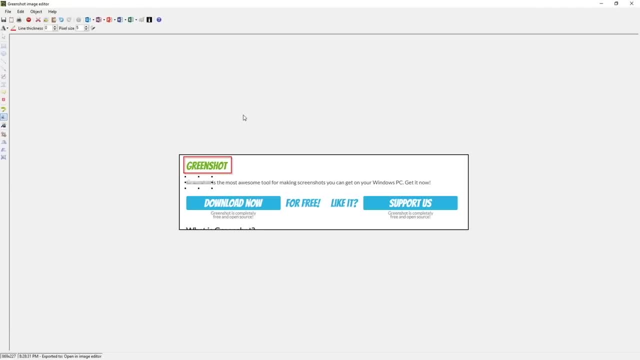 This is called GreenShot- Night of the ninth nut, Can't believe? I just said that. Anyway, it's called GreenShot. Basically, it just replaces your print screen feature, So instead of when you hit print screen, it allows you to drag and select. 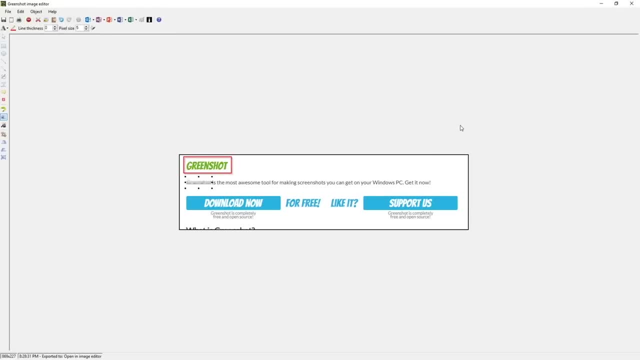 And then, if you wanted to actually do a print screen, there's like control print screen or something else that allows you to take a screenshot of the whole screen. Hey, thanks, Nate, That's awesome. So it looks like Flameshot works. 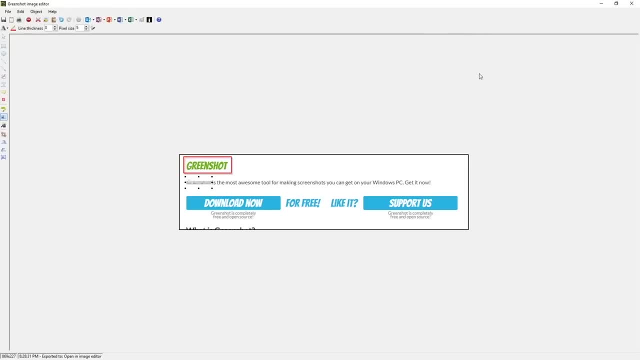 Yeah, some of you guys have some really good usernames. I'm digging it All right. So we are at 830.. We are really good schedule guys. So, in terms of notes like this is really what you want. You want a note. 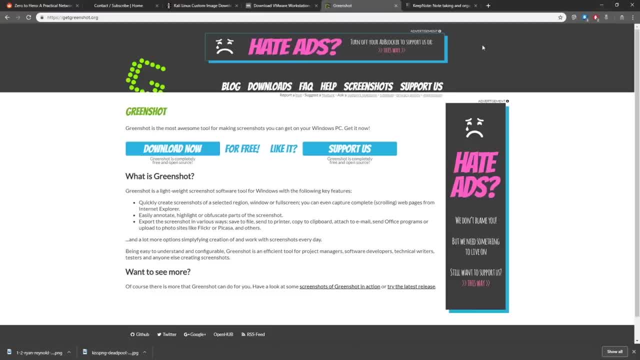 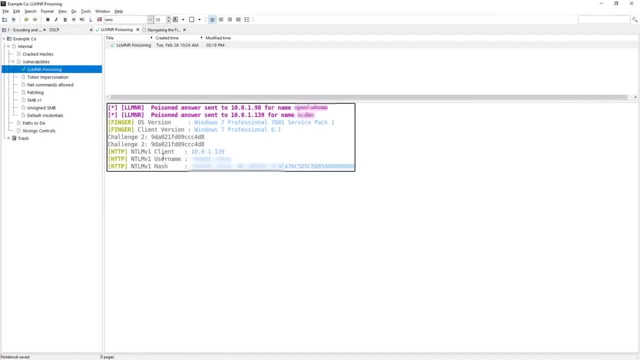 You want to show as much information in, like the screenshots that you can Like. if we go back into my keep note and we look back, like you want to see, like see how I highlight it, I got the. I can show that I've captured a hash or whatever. 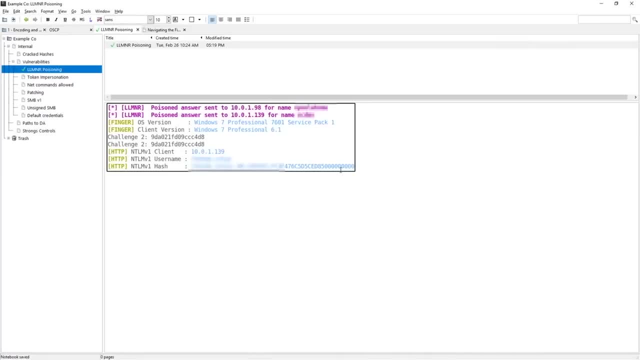 And a lot of times we'll blur this hash out That way, like: or if it's cracked, we'll blur the cracked part of the password out. That way, if we release a report, nobody knows what the password was. Same thing with like token impersonation. 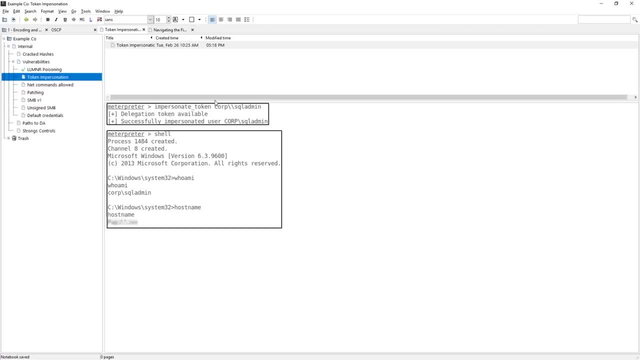 You want as much information as possible in these So Really cool stuff, And that's really it. So just as much detail as you can get as possible, because as a pen tester, you may have to go back and rely on your notes, and your notes are everything. 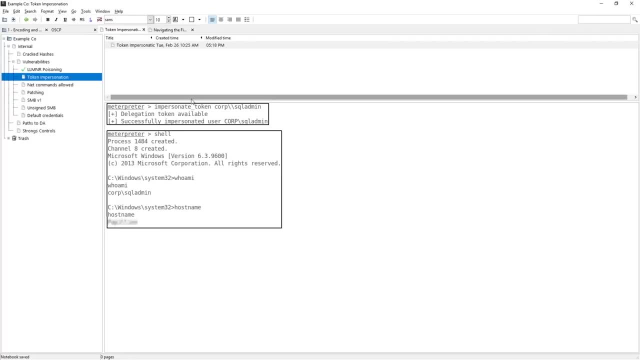 So if you're on an assessment and you're on site and you only have so much time on site if you didn't take a note or a screenshot or you know the right kind of things that you needed, and you go back to write your report and you're going to say, hey, I needed that. 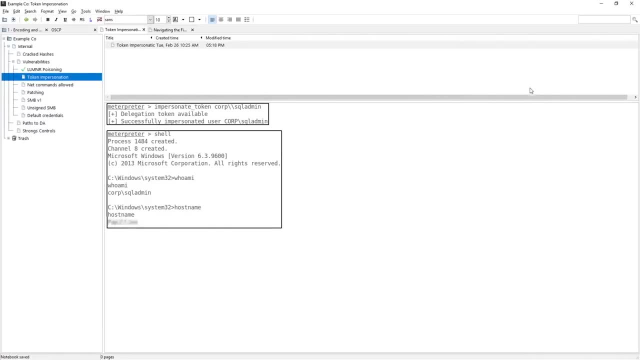 Well, you're screwed. You either have to go back on site, You have to somehow ask the customer, and they figure out that you messed up somehow One way or another, Right. So good call on the flame shot: I've never heard of it, but I'll have to check it out. 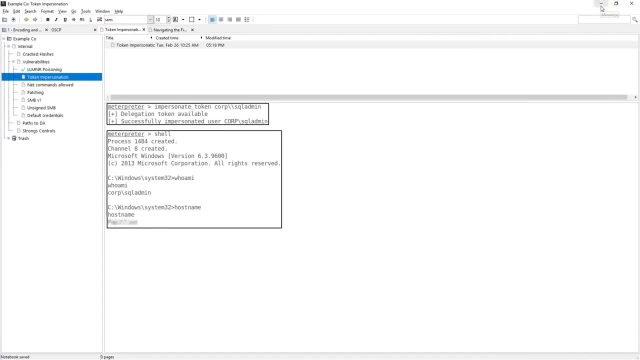 Looks like it's pretty good, All right, So I'm going to take a quick sip here of my lovely beer, and then we are going to dive right into Linux. So I do recommend that you take notes if I go too fast. This does have VOD for you guys. 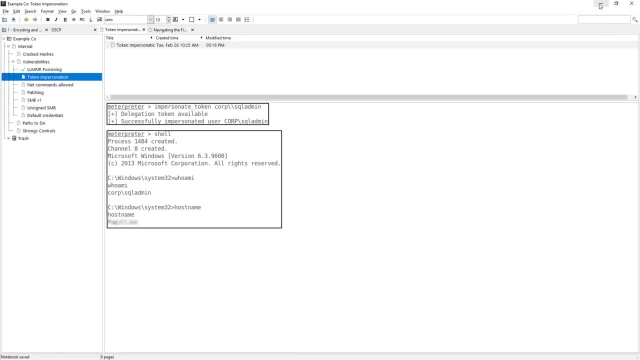 I'm going to try to talk slower. The notes are stored in a folder on the desktop Or wherever you save it, So they store into a folder and then into subfolders inside that folder. How much time do I spend on notes for the OSCP? 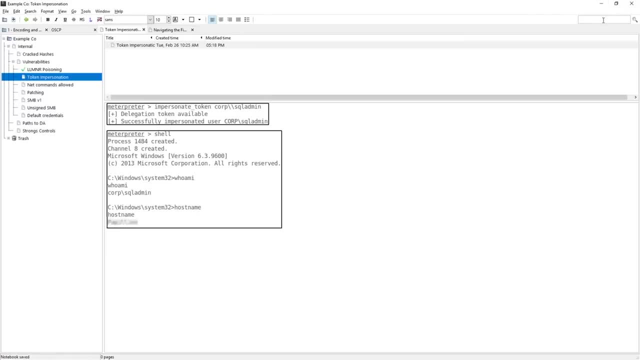 I got through the note guide, the lab guide, in seven days. My goal was to get it done in a week. Labs and exercises or whatever. For the most part there were some of them I couldn't get through that fast. Some of them you had to be in the labs to figure out for a little bit. 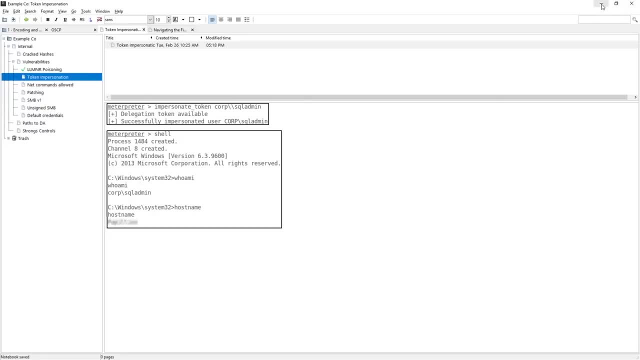 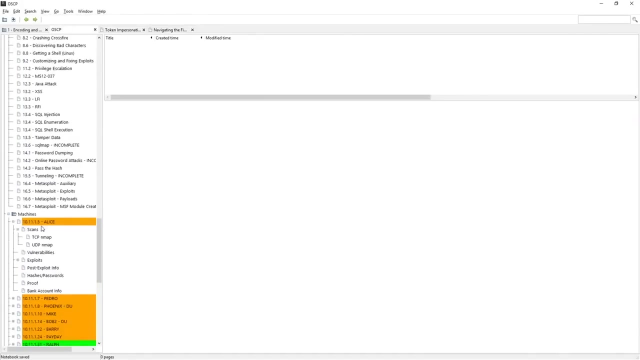 But that was seven days of work plus whatever you saw with the machines just was kind of as I went And those were a little bit different. Let me see if I can click in there without revealing too much information, So like, if you look like, say, this machine, this is well known. 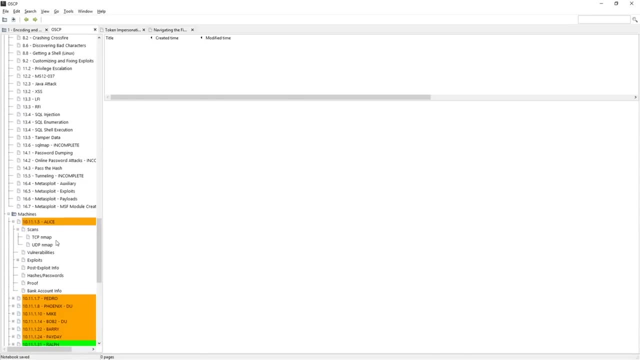 Okay, say, I had the machine number and the name. I did my scans- my TCP, my UDP. I had the vulnerabilities, I found the exploits, I found the information that I found post-exploit- Whether it was network information, valuable information, any hashes or passwords I found- and then proof pictures. 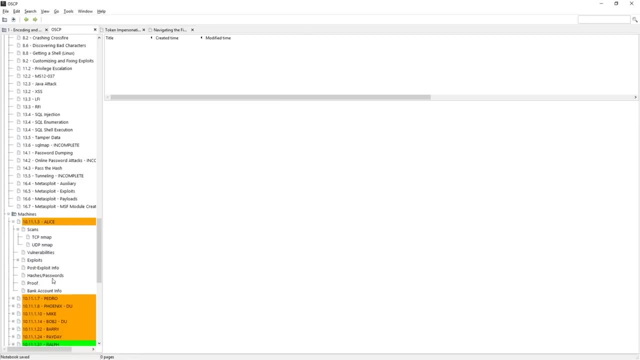 So you can see I really organized it out by machine too, because you never know when other things are going to come up. You don't know what machines are talking to other machines, And this is all kind of stuff we'll touch on and learn. 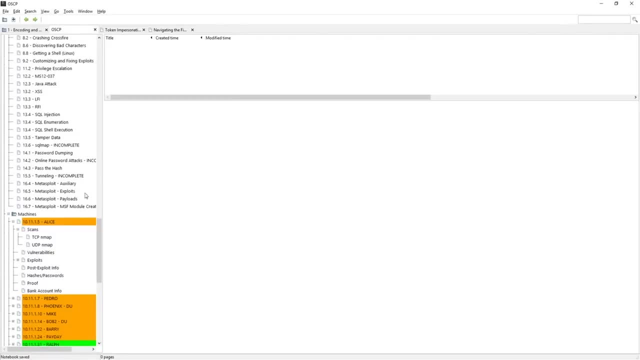 And I'll kind of guide you on how I want you taking notes as we go and get into this. But for the Linux section you really don't need that as much. It's just kind of going to be by hand and taking notes as you go. 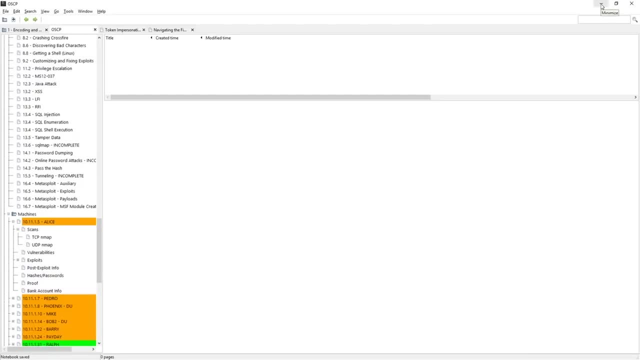 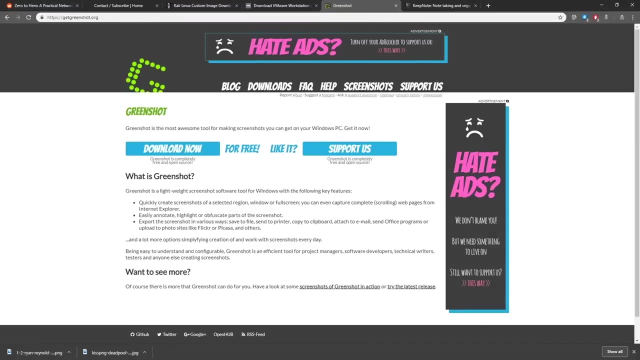 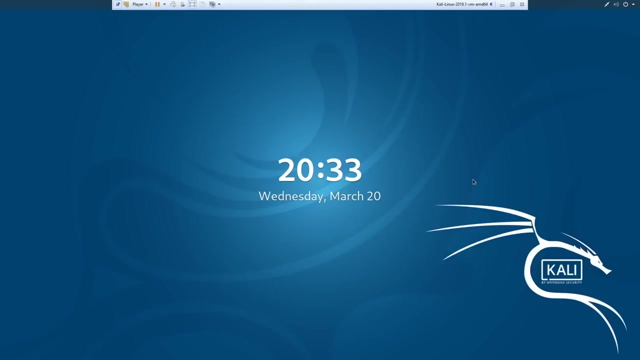 If you find something interesting. Find something interesting that you don't know And then watching it later. if you really are new to Linux, You guys are getting rich over here, Okay, so let's go ahead and hop right into Kali. I like VMing on Kali. 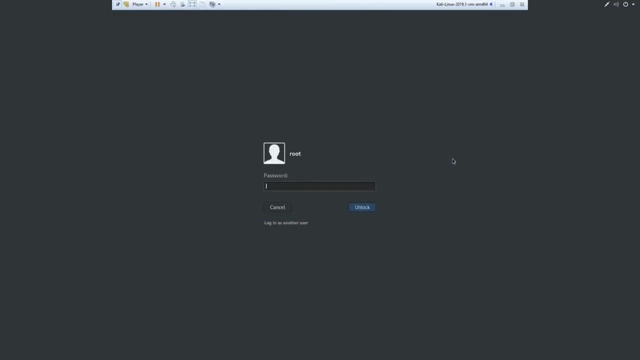 We have machines that we use like laptops, that we use Just specifically for Kali for work. If you want to go that route, you're more than welcome to go that route. I just I like having a VM for like pen testing. 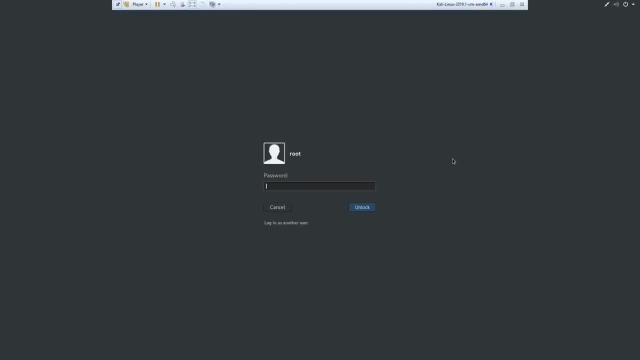 And it's more flexible, because there's some things that you want to run in Windows, Some things you want to run in Linux. You know, for me it's about flexibility, But for some people, you know, everything can be done through Kali. 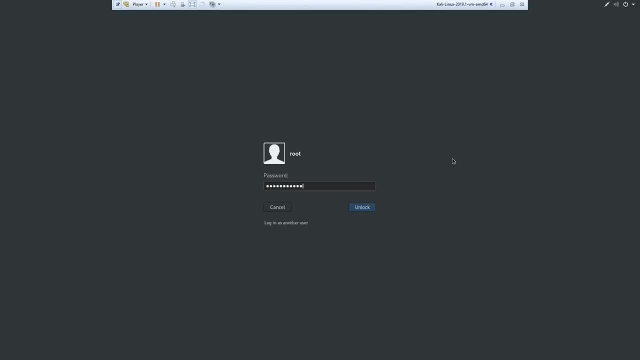 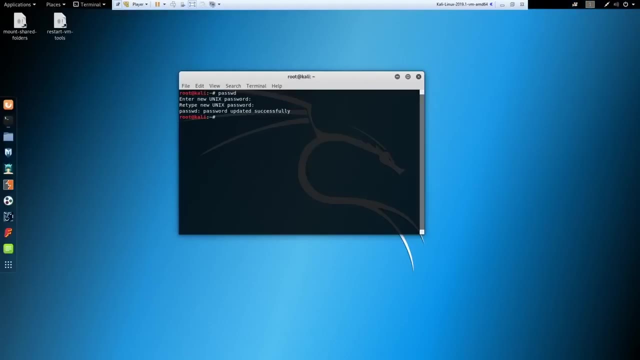 So let's log back in. All right, Let me get my notes up, Because there's no way I'm going to remember everything I want to teach you guys. That sounds like a lot of work. Red Finale: I like my distribution. Because Kali just comes with everything prebuilt. I know some people that do that. I just don't like doing that. I know a lot of web app people that do that specifically. They'll just install the tools they need on a distribution. 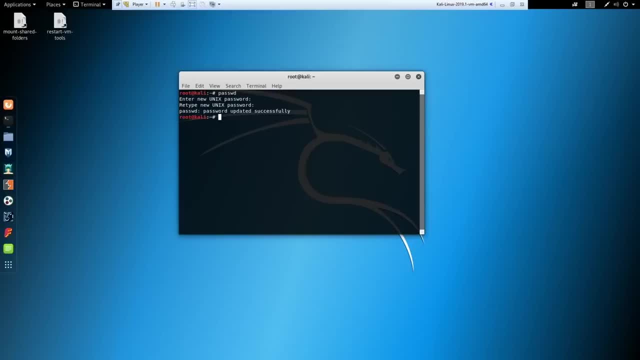 And you never know what you're going to need. So I'd rather just have everything instead of having you know the tools I like. All right, So what we're going to do in here is we're going to talk about navigating the file system now. 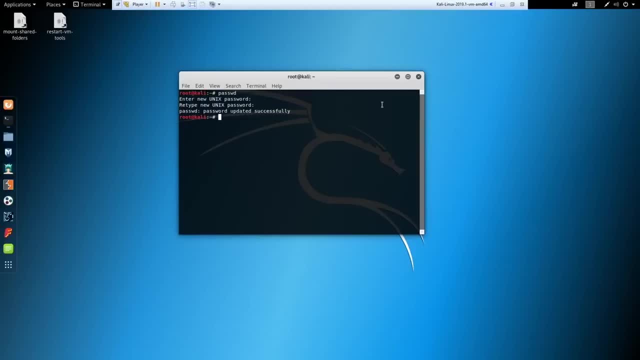 So all this is going to be about is how to get around, how to look at files and how to, you know, find files. So the first command I'm going to show you is pwd, which stands for print working directory. So what this means is it just says, hey, print. where I'm at. 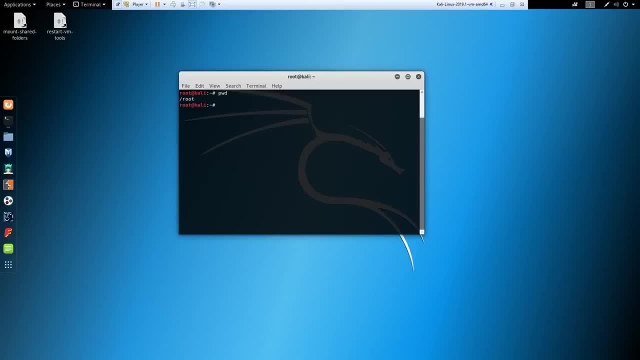 What's the location I'm at. You see, right now we're in the root folder. Okay, So if we want to move to a folder, we can use that with something called cd. So that's change directory. So if we want to change directory, well how do we know where we can go? 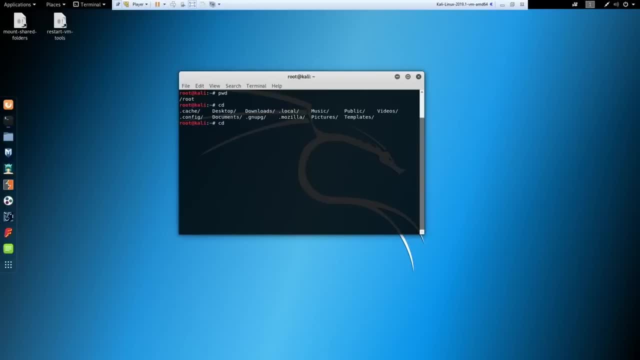 We can hit tab twice and see where we can go. We can change to out of this folder and that will give us some ideas, right? So okay, let's say we want to go to desktop, So we say cd desktop. 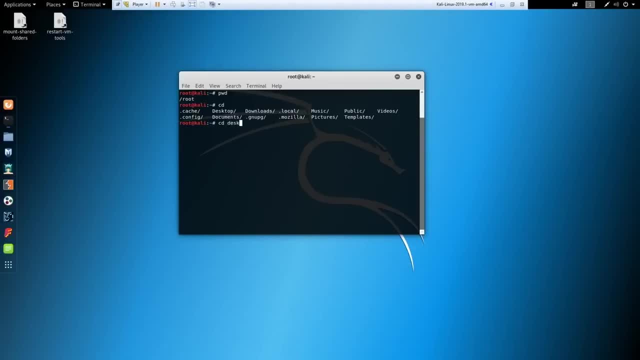 Now, if I start just typing in desktop and I try to hit tab to complete, it doesn't work because Linux is actually case sensitive, So we have to type it like that. But you can use tab to complete. See, I have desk. 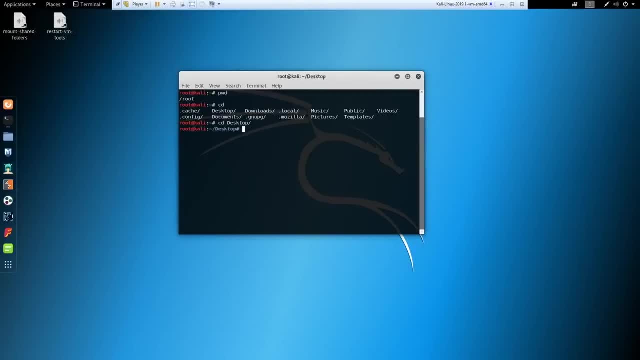 I hit tab and it auto completes. So if we hit enter here, you could see now that things have changed. And actually let me make this a little bit bigger. Let me see if the plus works. It never does for me. 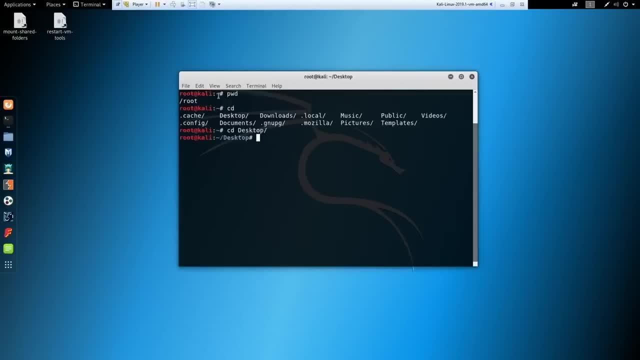 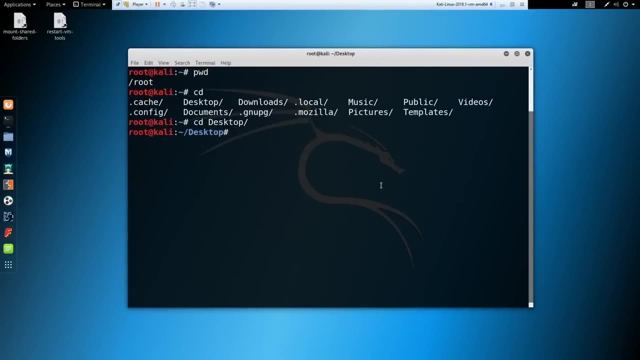 Okay, That way you guys can see. So now you can see that we're in desktop here And if we wanted to go back a directory we could say cd dot, dot. Okay, And now we're back into this little a tilde right here, which is our root folder, right? 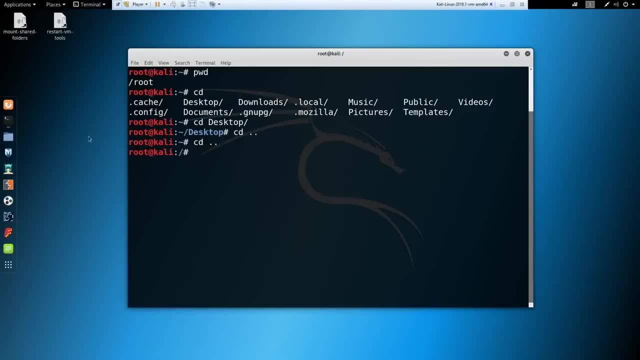 And if we try to cd dot dot again, okay, we go into like this forward slash of a folder. It's like a base folder for us. Now, if we cd dot dot one more time, we don't go anywhere. So we are in the lowest that we can go in terms of a directory, right. 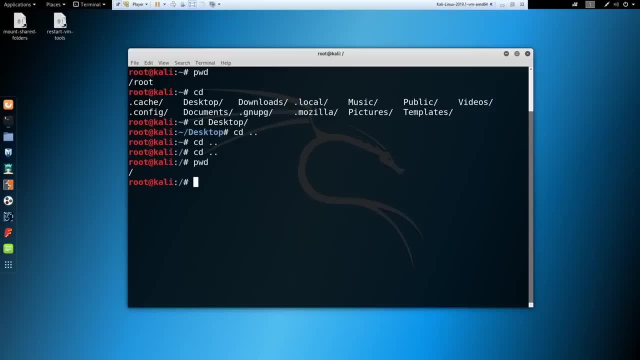 From here we can actually say: okay, how do we see what's actually in this folder? Well, we could do a tool called LS, which stands for list, And we're going to say LS. Okay, So in this LS we see that we have some files, it looks like, and some folders here. 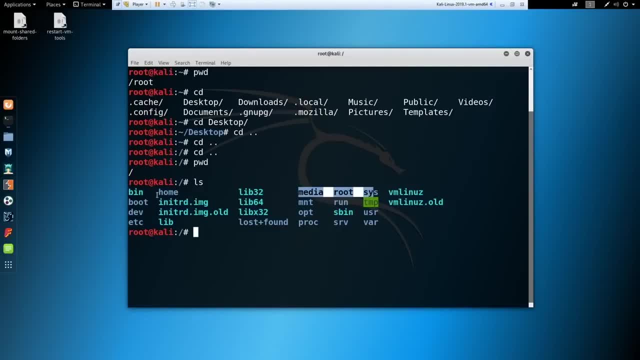 We've got a home folder- media root sys- And we could try to go into these, So say we want to go into home. We could say cd home, like that We'll go right back into our home folder. We could say LS in here. 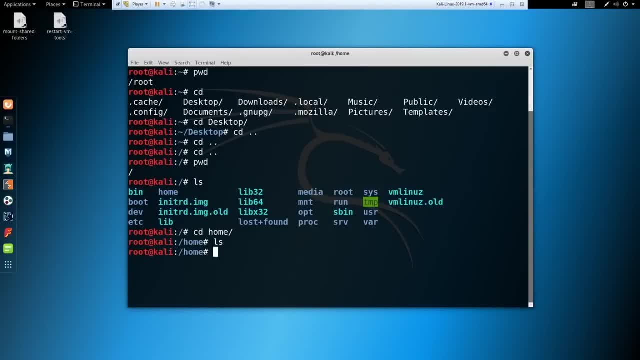 And there's nothing in the home folder. So from here, what we can do is we can actually also use change directory from outside of the folder that we're in. So right now we're in the home folder, right? But say that we wanted to go into the root folder that we were in originally. 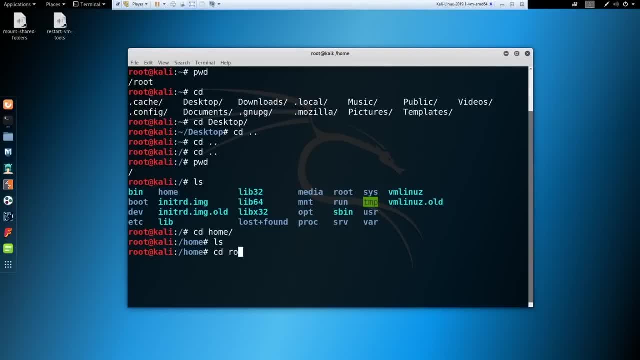 See this root folder. Well, if I start typing in cd root and I autocomplete here, it's just not working. Well, that's because we'd actually have to put a forward slash in front of it, because we're going to call it cd root. 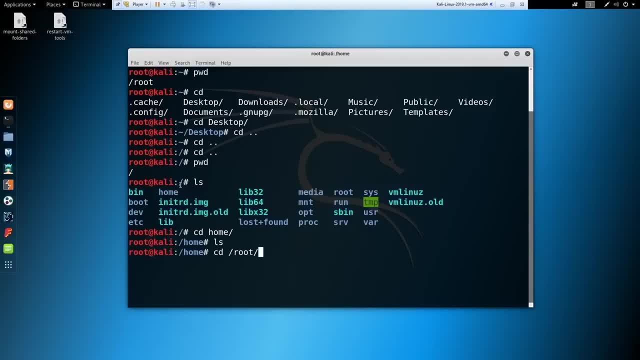 Because we're going to call it from where it actually is. It's in this base folder of a forward slash And then we're going into root So we can change directory and call directories from locations other than where we were at. So right now we're in root. 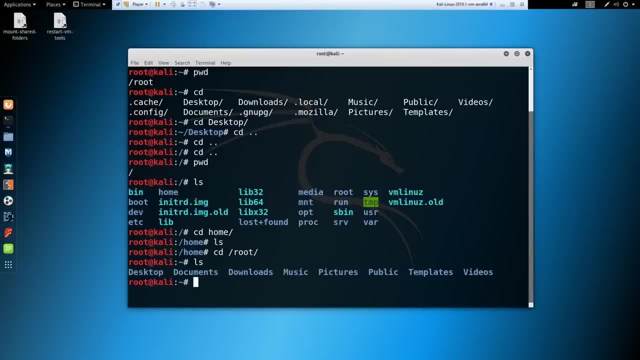 And if we ls, okay, we have all these folders here, desktop documents, etc. Again, with ls, we don't have to be in the location that we need to be in, So we could say: ls desktop And it'll ls what's actually in the desktop from where we're at. 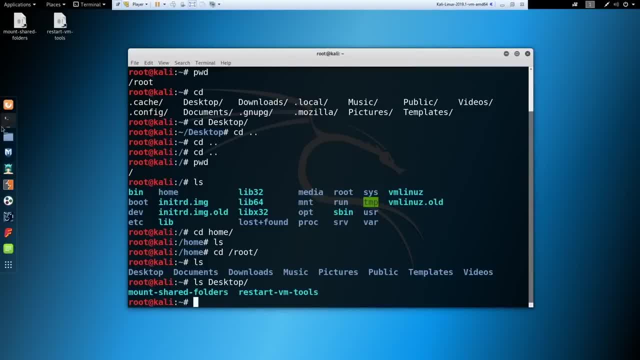 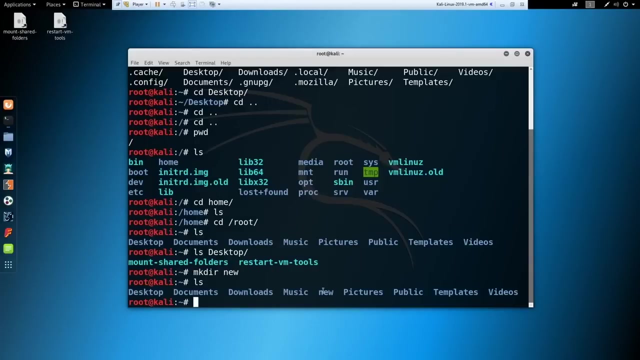 Okay. So the next thing I want to show you with this is the make directory and remove directory features. So we can say: we want to make a directory, Let's just call this new, Say make dir new, And if we say ls, you could see that the new folder has been added. 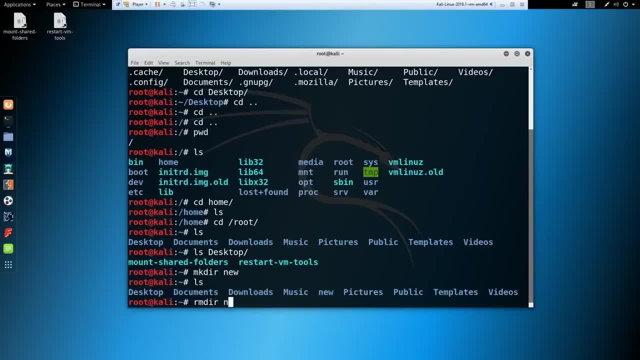 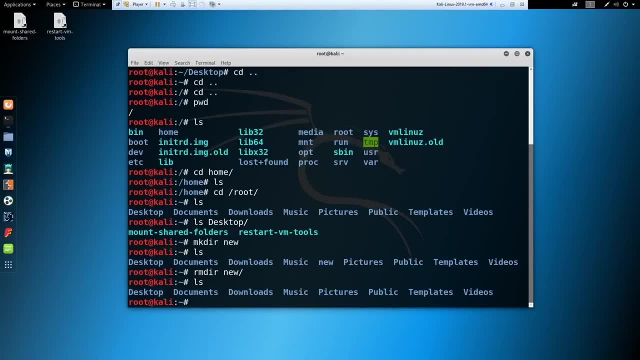 And then if we say remove directory new, we say ls, you could see that that new folder has actually been removed. So easy way to make a directory and remove a directory. And if we look in here there's another thing we can do. that's a trick. 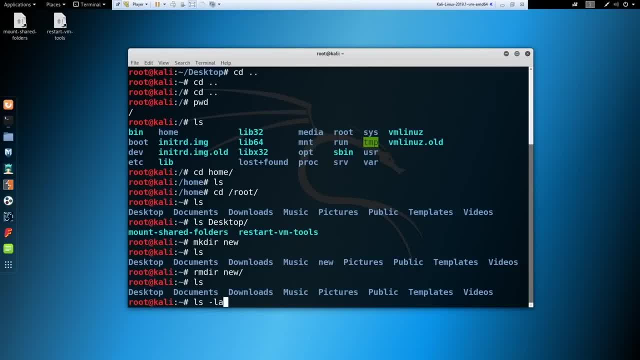 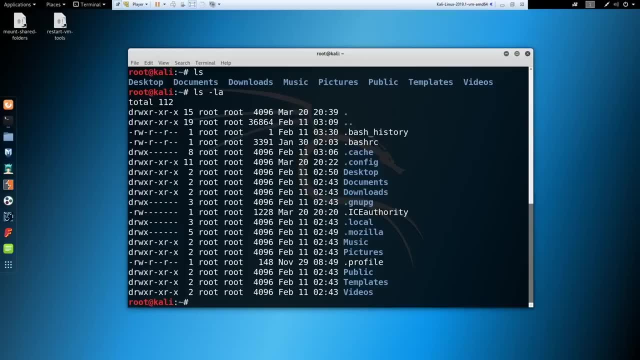 And we can say ls, but we can actually say dash la, where it lists all. Now, this is really interesting And we're going to cover this a little bit here in a couple minutes. So when we look at ls la, You could see that there's some stuff in here that we actually never saw. 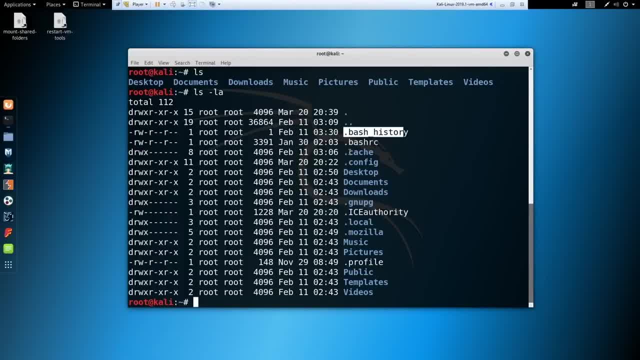 All these dots that are in front of these files or these folders. Well, those are actually a hidden file, right? So we didn't see them with the normal ls, But we did see them with an ls dash la. So if you're pen testing a Linux environment, it is always smart to try to say ls dash la. 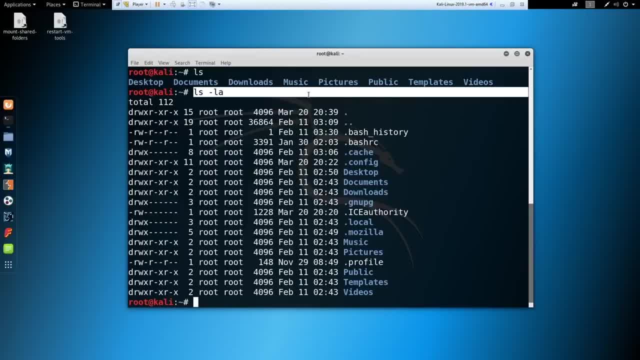 Because you never know what is hidden or what you might be missing, And that goes especially for calculus. You might want to capture the flag type things, Because sometimes they like to hide stuff on you in really, really basic locations. So it's always worth a try to see what's going on in here. 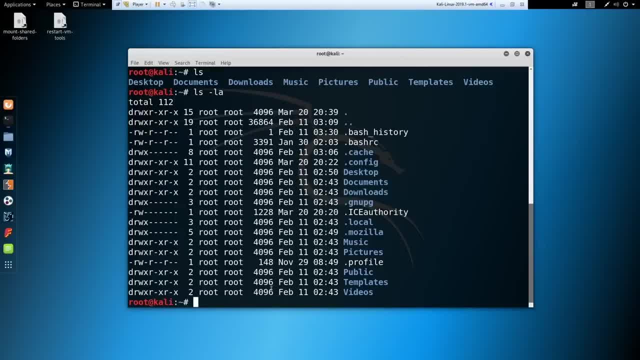 Okay, So from there, when we talk about navigating the directories, one thing we can do is we can copy, remove and move files. So I'm going to say echo, hello, And I'm going to put that into a new file. 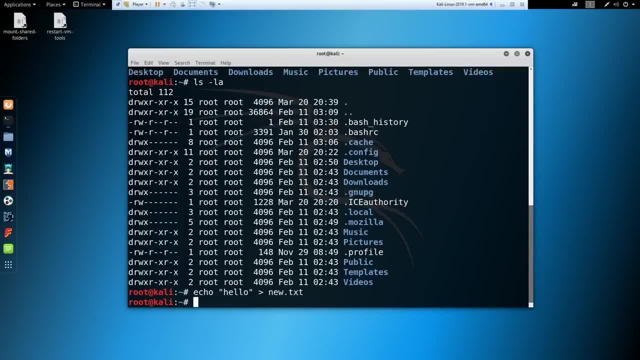 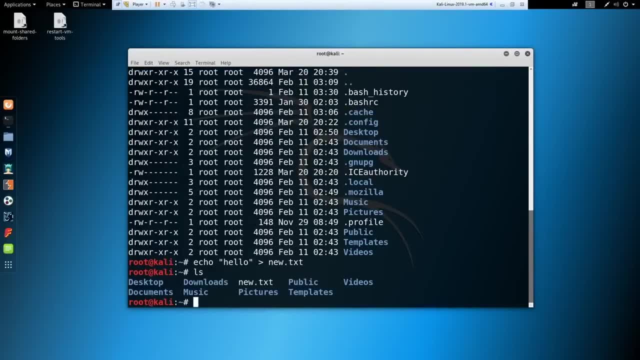 We'll just call it newtxt And we'll cover how to make new files in a little bit. So if we say ls, you can see that newtxt is here And I just want to copy this file. So if we copy this file, we can copy newtxt and we can place it wherever we want. 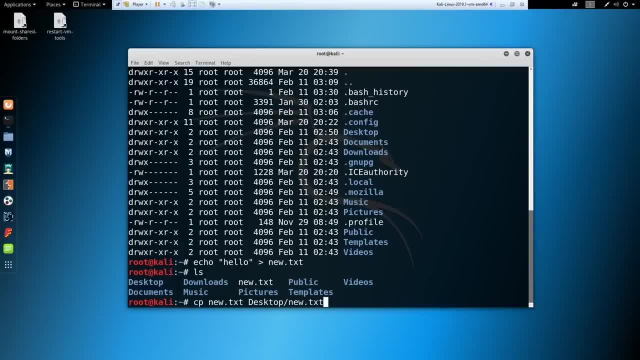 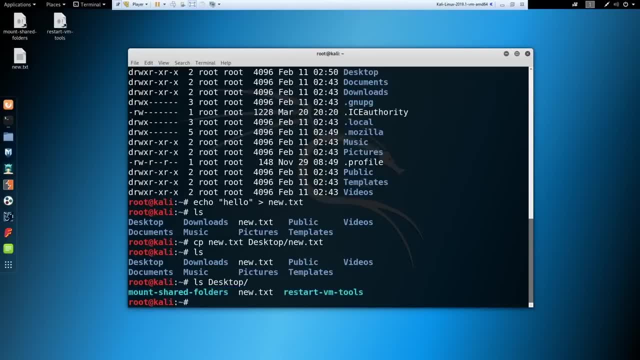 Let's say we want to place it on the desktop, We'll call it newtxt there. So if we lstxt, So if we ls, you can see that newtxt is still here. But if we ls the desktop, you can see that newtxt is there as well. 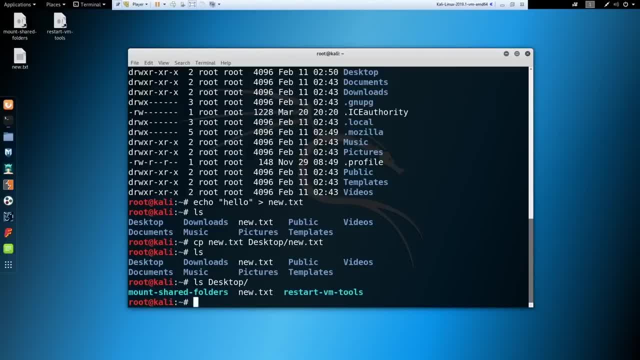 So what copy does is creates a copy. Now let's go ahead and remove the file from the desktop. And again, remember we don't have to be in the directory that we're in. So let's go ahead and remove desktop newtxt. 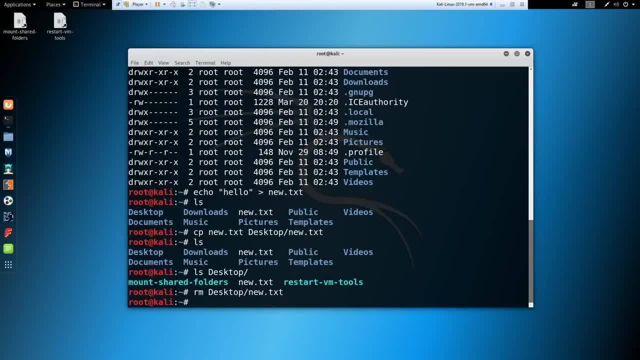 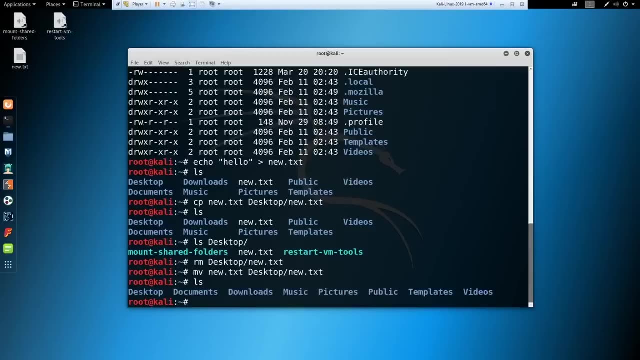 Okay, So that's how you remove a file. is rm. Now, if you want to move a file as opposed to copy a file, you could say: move mv newtxt into desktop newtxt, And if we ls here, we see that that's gone. 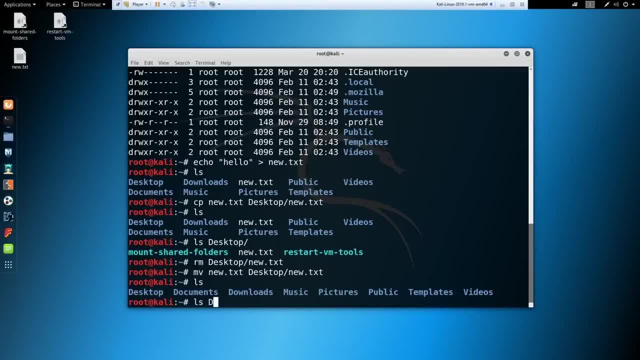 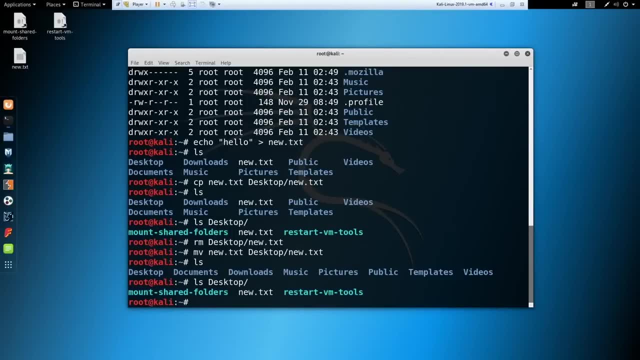 And if you saw my desktop, you saw it came up. But if we ls the desktop, newtxt is there. So a nifty little trick. I want to remove that newtxt file again. If you hit the up arrow a couple times, you could see where we actually removed it from the desktop. 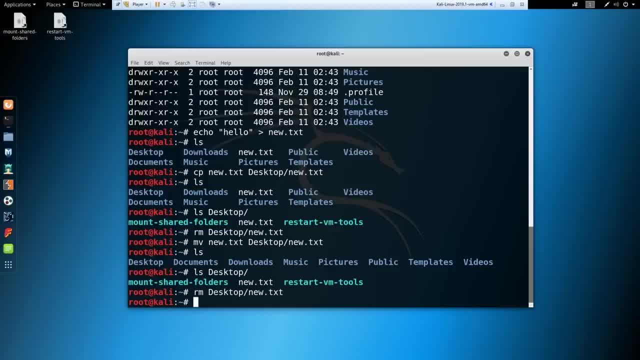 I'm just going to run that same command again And there we go, It's gone. So a couple things that I want to do here. I want to create a new file Again. I'm going to create this same echo: hello, newtxt. 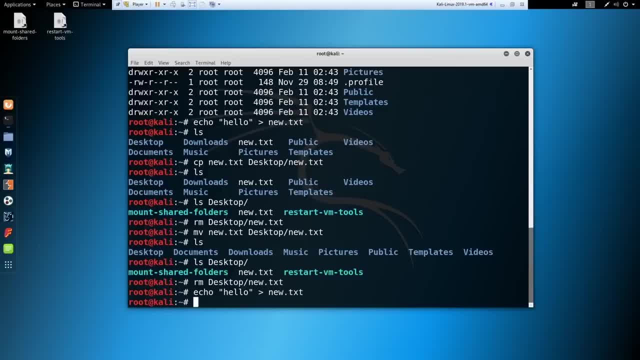 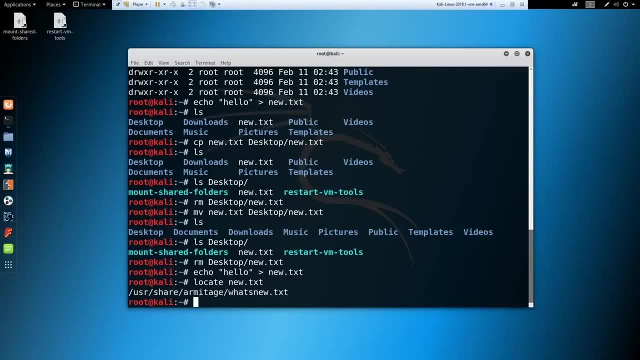 And I want to find that file. So I say: locate newtxt. Okay, Well, I found that what's newtxt, But that's not the file we're really looking for. Okay, So what we need to do Is we actually need to occasionally run this command. 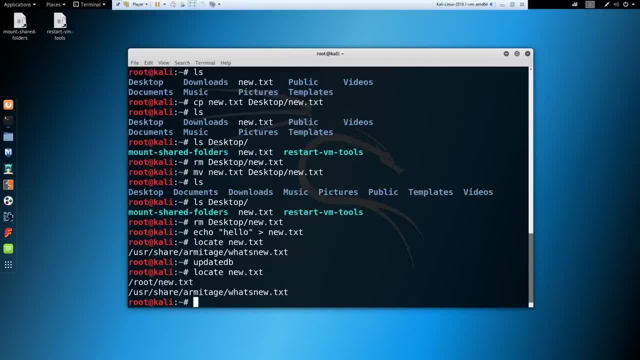 It's called update db. You're updating the database. Let's try it again. Aha, So now it shows up. So any new files or folders that come up, we might need to run update database to see where they're at. 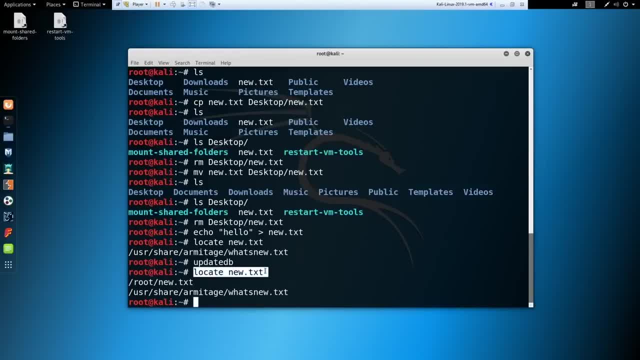 But now we can just use that locate command to quickly find a file that we're looking for. So we've already actually covered the password command, So I'm going to go ahead and skip that. And the last command in this section of navigating the file section. 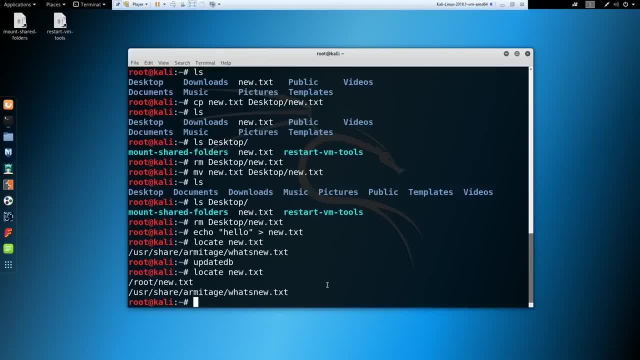 Of navigating the file system that I want to show you is important Outside of Google being your best friend. Google is always your best friend, But if you need something quick and dirty, man is going to be your second best friend. So you say man which stands for manual. 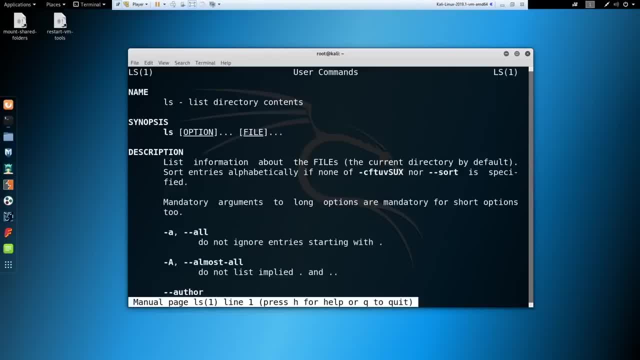 And we'll say: man ls. Let's look up the ls command And we come in here And we say: okay, It tells us the name, which is ls. This is going to list directory contents. It gives us the description, the synopsis. 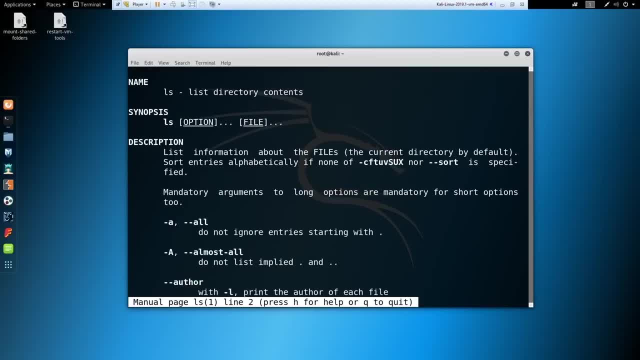 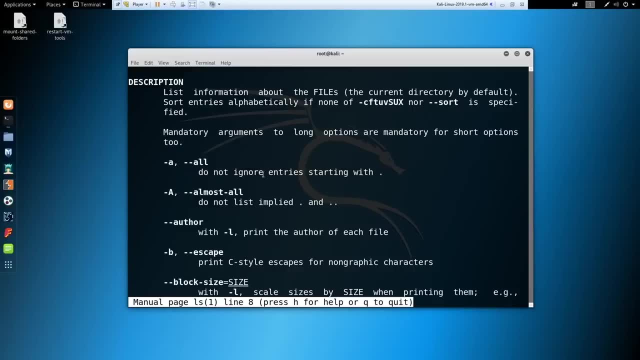 And it says: okay, what do some of these entries do? So we can kind of scroll down and look through these and see what they do. So remember, we did a dash a earlier. Well, that stands for all. And it says: do not ignore entries starting with a period. 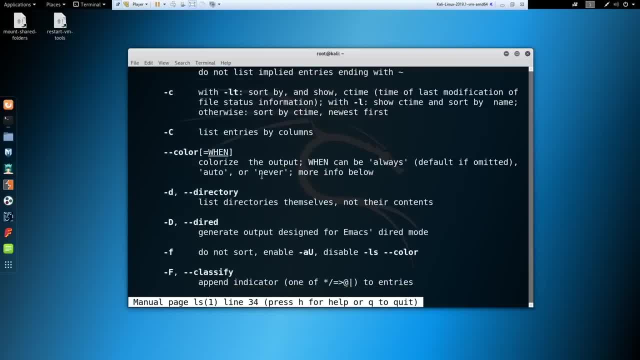 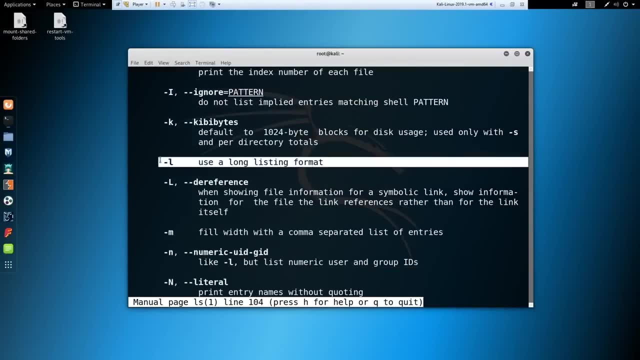 Remember those are our hidden files. Okay, So let's look at what the l stands for. Okay, So it says: use a long listing format. Remember the things that were off to the left? that was kind of all jumbled together. That is the long listing format. 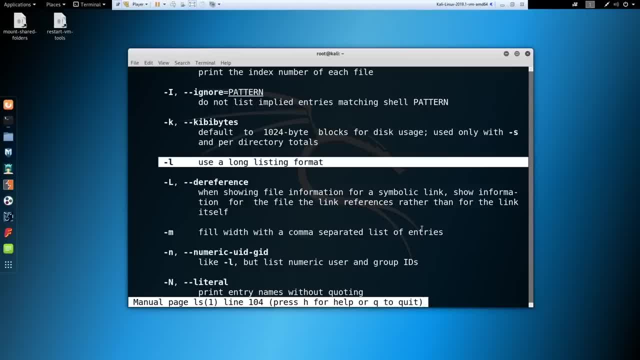 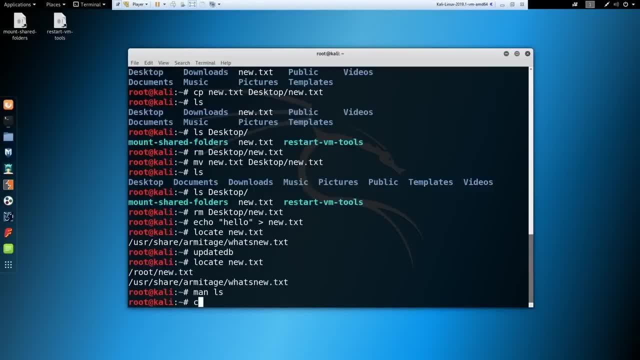 And we're going to talk about that in just a second here. Actually, we're going to go right into that now. So when we talk about the long listing format, if we come in here and let's go to the desktop, actually, 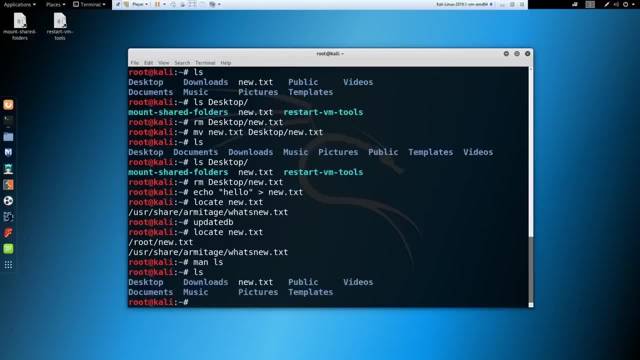 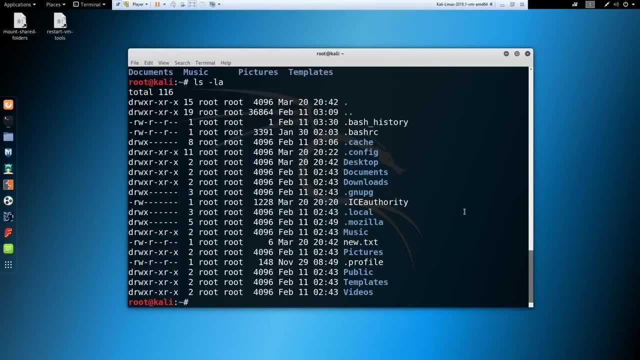 No, we're here. I lied, Okay. So we've got the newtxt file that we created, Let's say ls-la again, And we'll look through this. So you see, here there is all this jumbled mess over here. 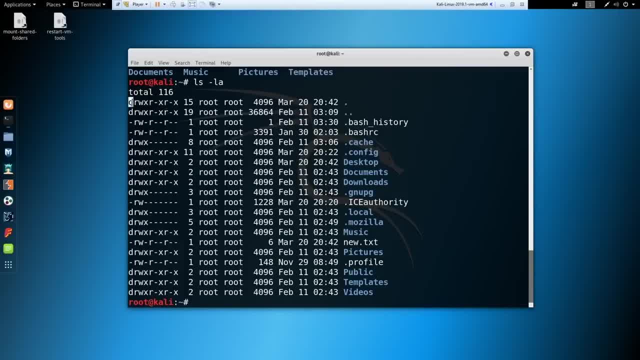 So when we talk about this first row, this first line here, this first letter, this d stands for directory. So if it has a d in front of it, it's a directory. It's also color coded, so blue is a directory. 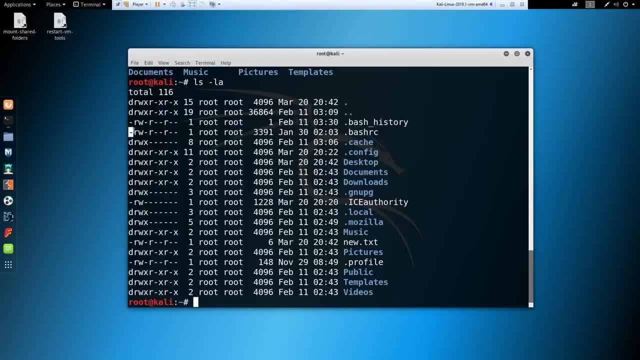 And if you are seeing a dash in the front, that's actually a file. So you can see this newtxt that we created is sitting here as a file. And then you're actually broken down into three groups here, where the term rwx stands for read, write, execute, 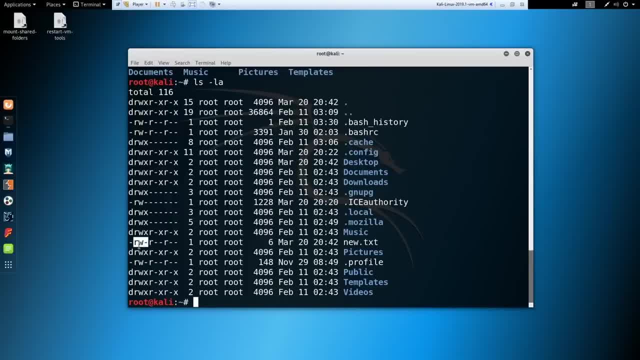 So we have three options set up here. If it's switched on, it'll show, If it's switched off, it'll be a dash. So if you look at the file newtxt, you can see it's read, write, but not executable. 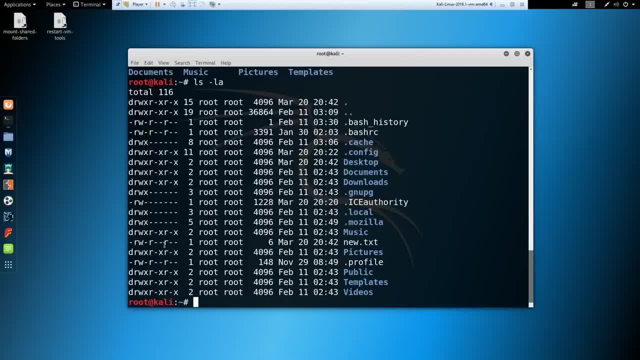 And then here it's read, And then here it's read. So these three groups, this first group here, this is the file or folder owner. The second group here is the group owner, And then we have all of their permissions. So if you're the file owner, which, as I said, is the folder owner- 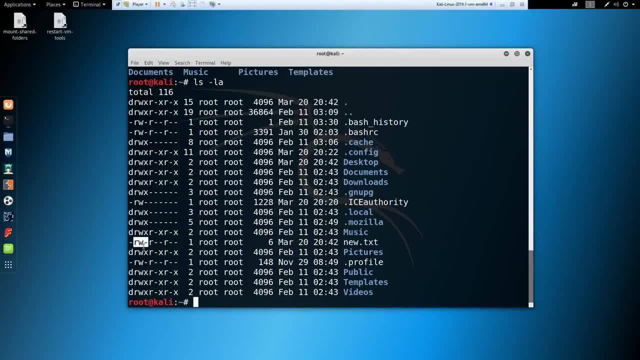 And then if you're the file owner, which is this root we are. these are the permissions we have Right now. we can read the file and write the file, but we can't execute. If I create a new account for, say, Bob, then Bob would come in here and Bob only has read access. 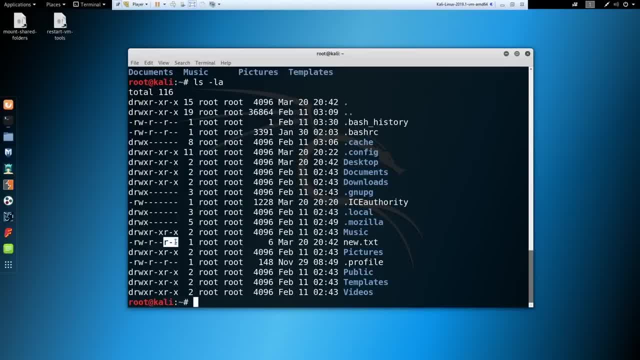 He can't write to this file or do anything because he's not the file owner, unless we put him into a group or made him the file owner. So now, what we can do with this is we can actually use something called chmod, which stands for change mode. 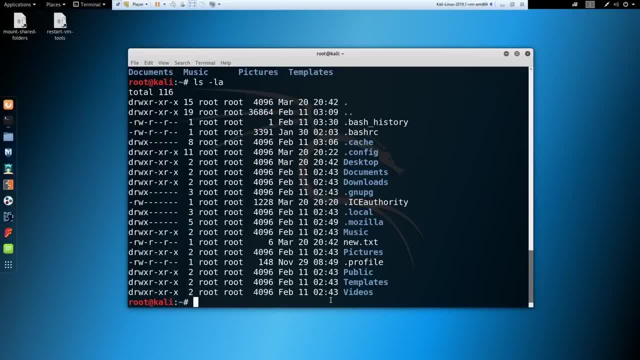 Now there's a couple different ways we can do this. So there's a numbering system. We could say: change mode 777.. Now 777 on newtxt will give it read, write, execute for every single thing. I don't like really doing that unless we have to, but I do like using this instead. 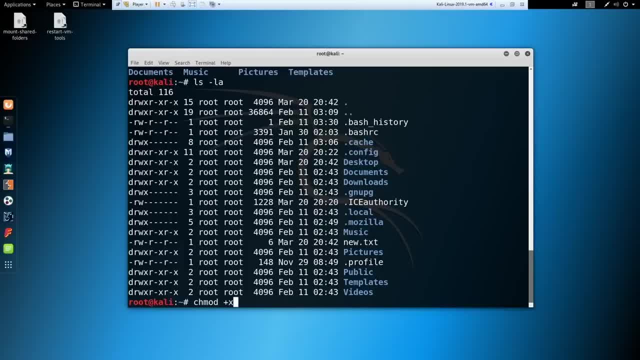 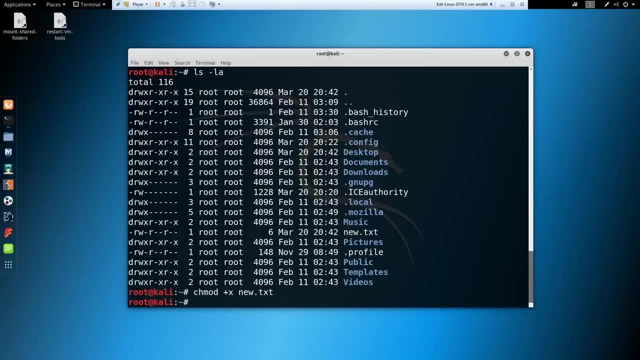 I like using plus x. This means we can use execute on that file. So let's say newtxt with execute, And then you come into here and you say, Okay, well, it's ls-la again and it turns a shiny green. 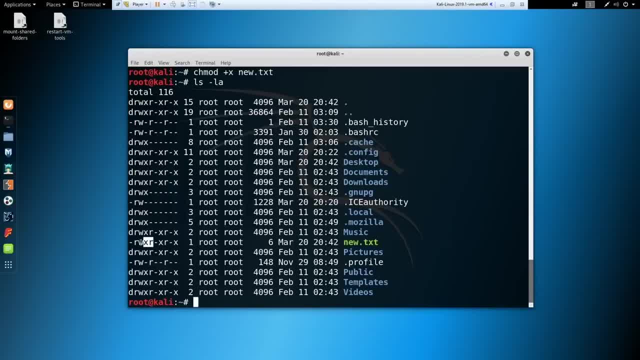 That means that it's executable, And that gave that permission, not to just me, but it gave it to everybody. So what we do here is, when we're using this, execute. this comes into importance when we're trying to write our own scripts or we're trying to use other people's scripts that we download or we're trying to run an exploit. 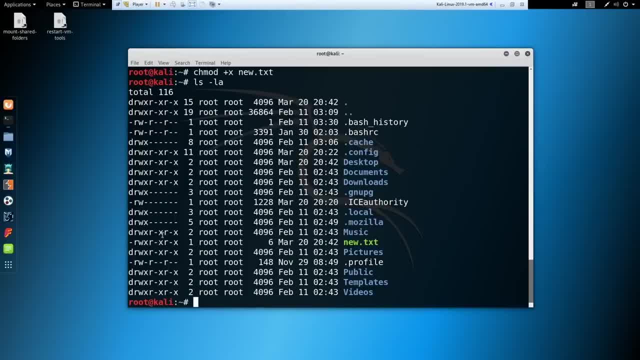 Later on in the course you'll see really its importance. But we need to have a file executable because if we make a script- and I'll actually show you in this lesson why it's important a little bit later- what you do is you have to have it executable in order to execute it. 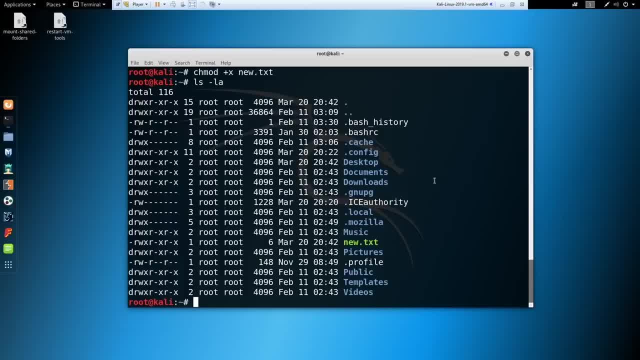 If that makes sense, it should. So if you try to run, like, say, a bash script and it wasn't executable, it's going to say: hey, I don't know what you're talking about, Can't run this right now. 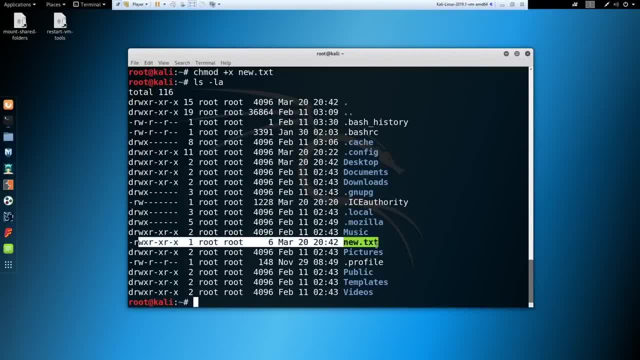 So very important. when we want to run a script or Python or whatever we're doing, that we need it to be executable. Okay, moving on, we're going to talk a little bit about users and some important files here as well. We're never covering the removeRF. 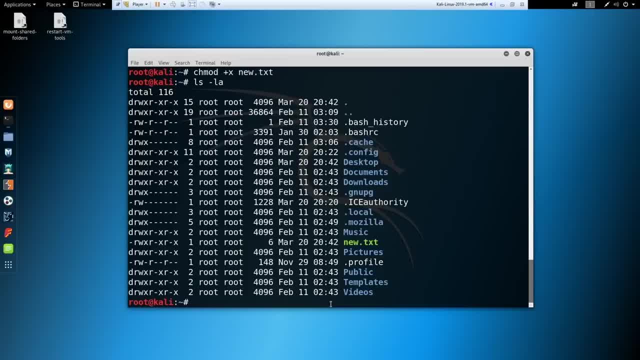 You're funny, That's the alt F4 times 100.. Anyway, so when we come into here, a few things I want to show you. So add user is the first thing I want to show you. So let's just say we want to add user. 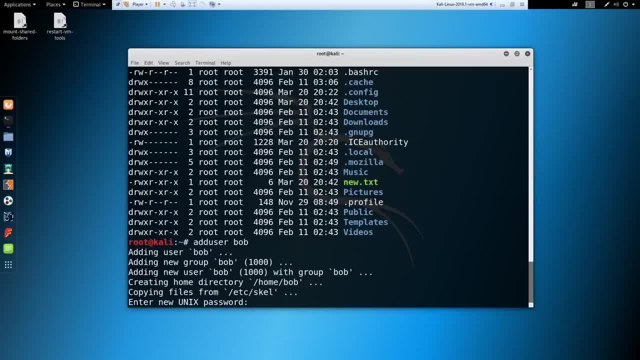 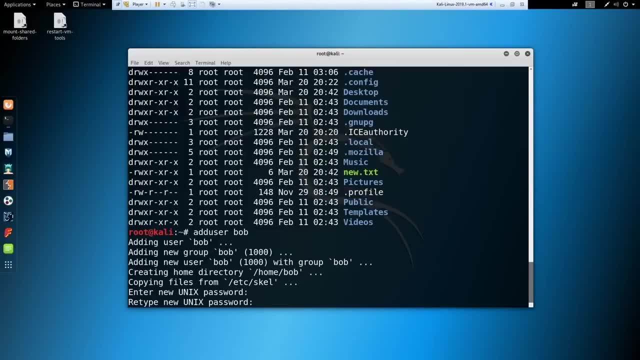 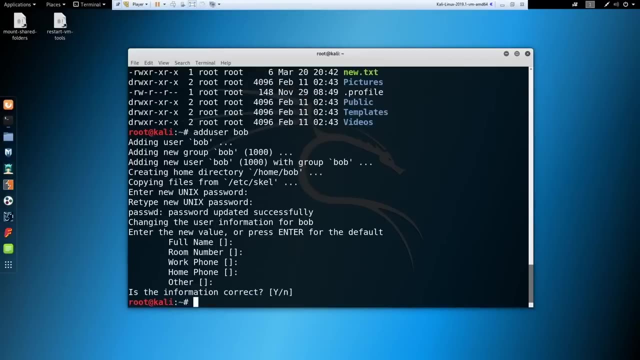 We'll call him Bob. Okay, we're making a guy named Bob. You can make Bob's password whatever you want, Okay, and then you come in here. You can enter information or not. Hit enter, Awesome. So let's look at Bob now. 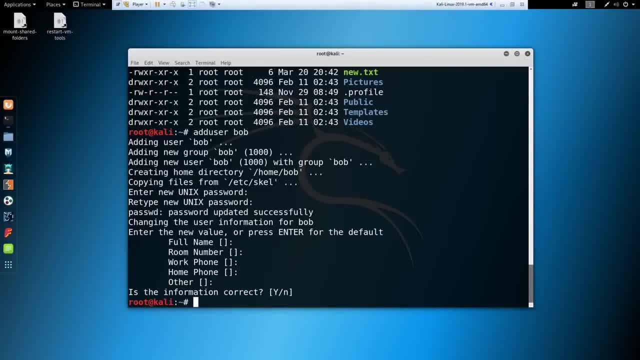 So if we come in here and we say, all right, what are some important files that deal with users- And you're going to be asked this on an interview- You're going to find this, you know, when it comes to just pen testing, 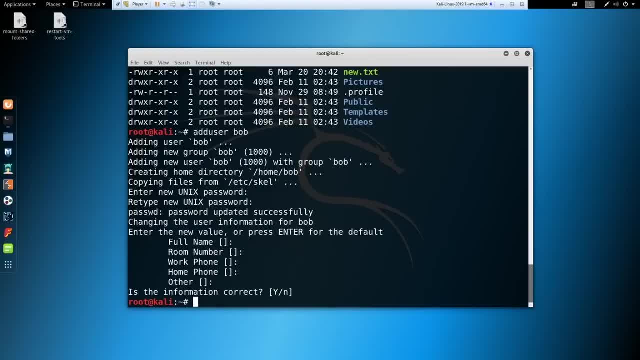 You're going to find this when it comes to capture the flag, A lot of times you're going to need to know these files right. So one of the most important files- and we're going to use a command called cat- is the Etsy password file. 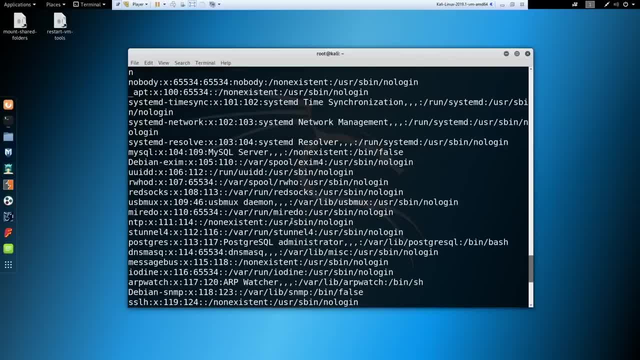 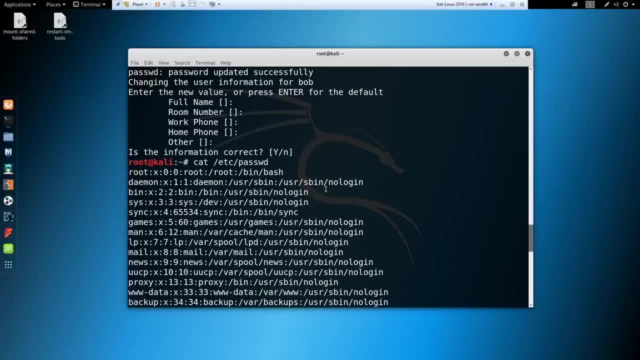 Now the Etsy password file is called the password file. Though it does not store passwords, It used to way, way, way back in the day, store a password. Now it provides a placeholder of an X for a different file called the shadow file. 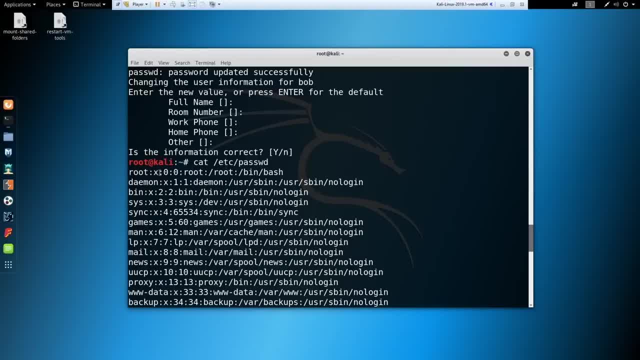 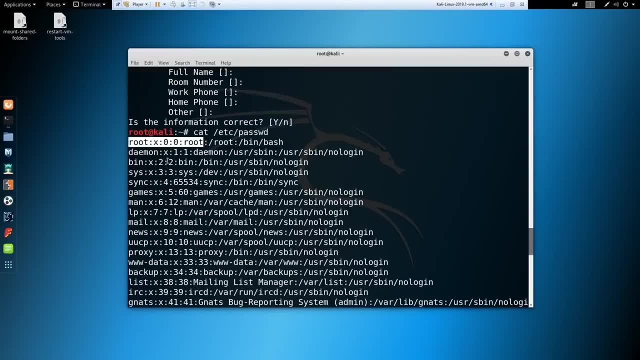 But you can come into here and you can see information, You can see who the users are, You can see that there's root And you can see what their UID is, et cetera. Well, if you scroll down, typically you get to the bottom. 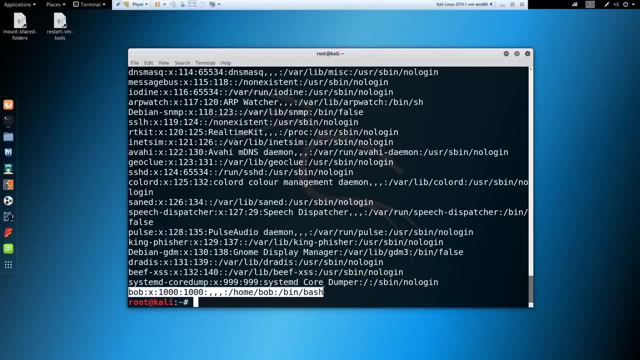 You find the users that are actually on the machine. They're actually on the machine as well, other than root. So when we talk about those users, we say, okay, well, we just created Bob Bob's in this group- 1,000.. 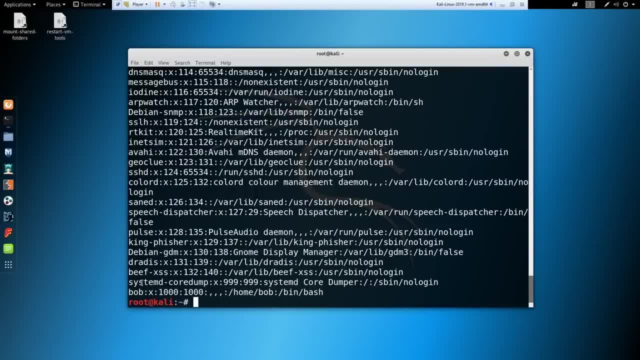 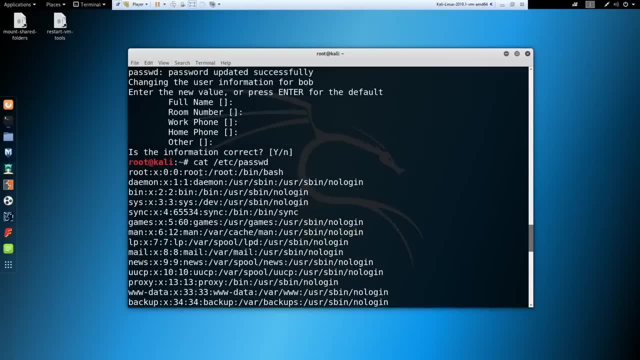 That's pretty standard And that's about that's all that's here. If we kind of look through this, these are all just kind of system user accounts that we really don't have a lot of interest in. We're really concerned with root when we're pen testing and we're really concerned with the users that we have for the most part. 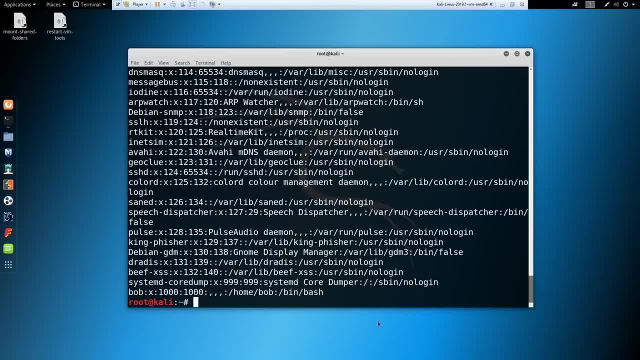 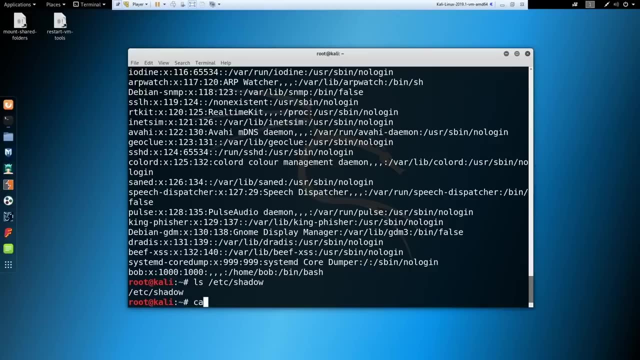 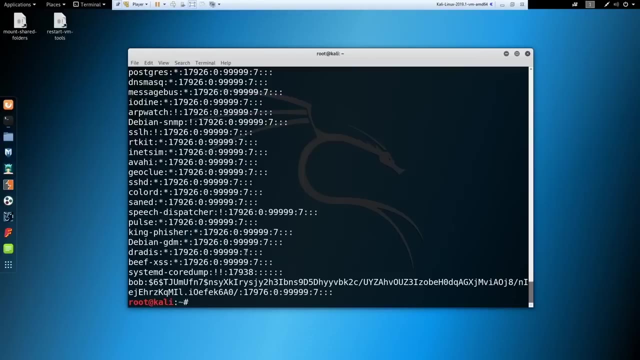 Especially when it comes to like capture the flag type stuff. So you can also say ls etsy shadow here And look at the shadow file And I said ls, I meant cat, I'm sorry, Spaced Okay, Yes, beef. 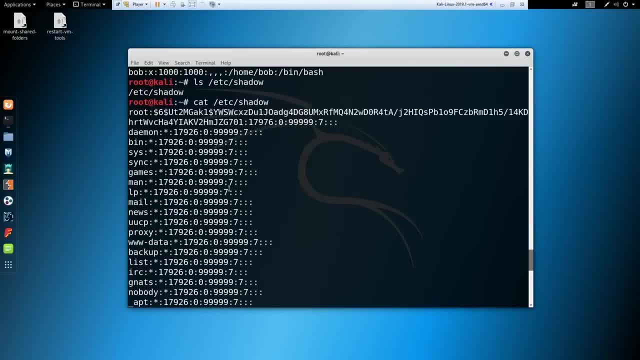 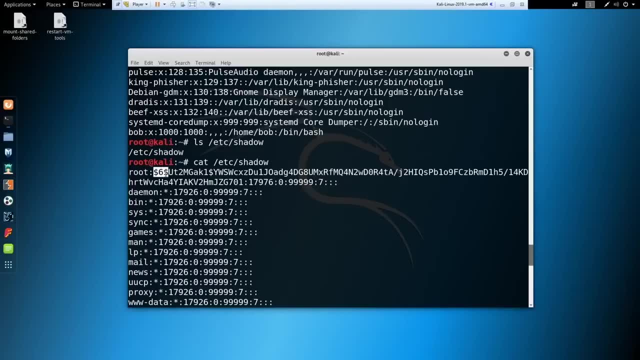 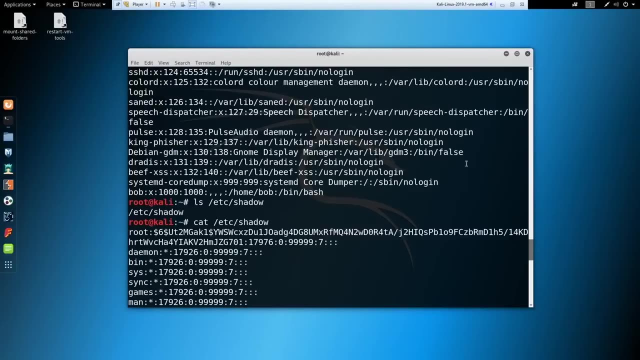 The hook, The hooker of the pen testing world is beef. Okay, You come in here, You see this hash right And you have this hash information. This is the no-no that you should never give access to right. This is the root. should only access and that's pretty much it. 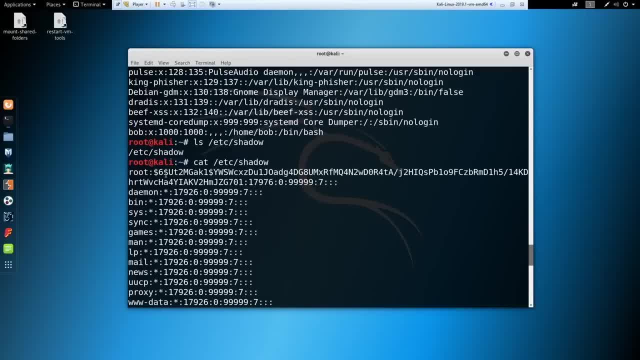 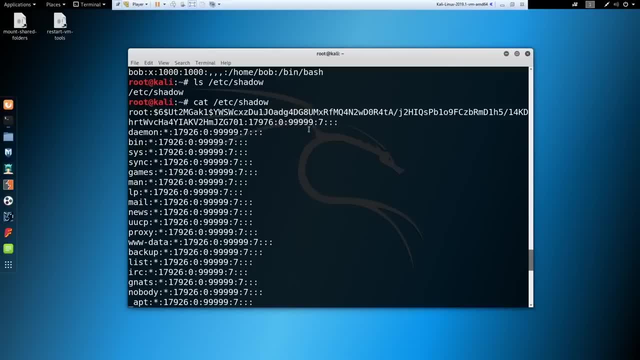 Because I've got the hash for Bob, I've got the hash for root here And we could in theory crack these hashes right And it would probably be pretty easy. So if I came into here and we can use a tool later on that I'll show you. 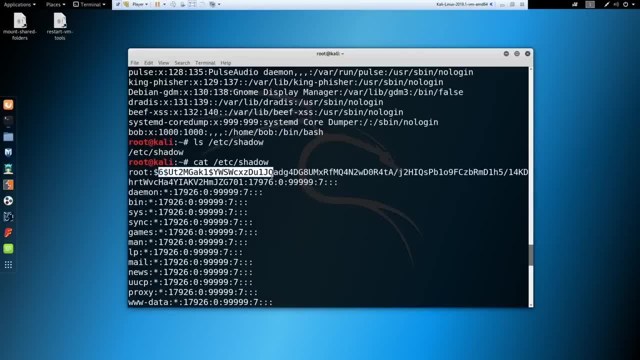 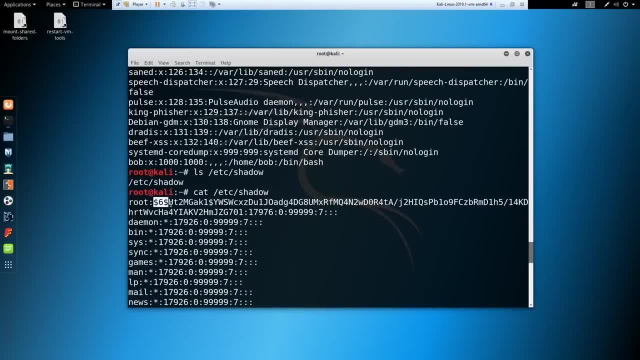 It's called unshadowing. Basically, you take this hash or this shadow file and this password file and you kind of combine them together. What it does is it takes the root, it places this hash in place of the x and then it runs the rest out into here. You can run that through John, or you can run that through Hashcat or whatever, and you can attempt to crack it. Does it have the salt listed with it? If it has the salt, it doesn't mean it can't be cracked. 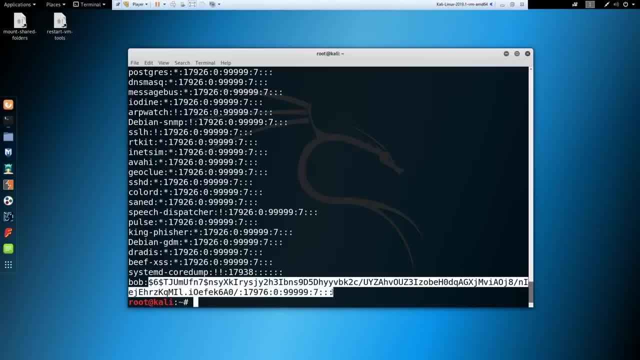 It's very- I mean, these ones are very well known and crackable. If we ran these through, I bet for Bob. I put Robert123 for his password, So I'm pretty sure you could crack that fairly easy with Hashcat and a decent password list. 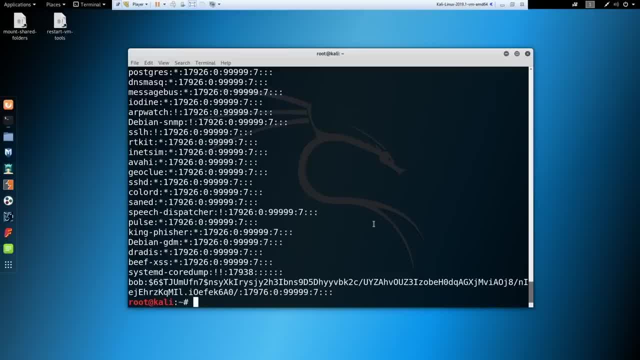 It knows the mechanism. There's a donate button. if you guys are really concerned with donating, There's Patreon and there's a donate button down below. If you're on a phone, it doesn't work out as easy. There's an info button if you're on the app. 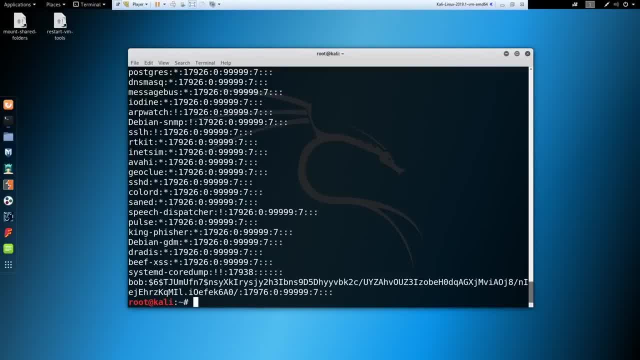 There you go. Yeah, there's the Streamlabs. donate. Thanks, guys. I really do appreciate that. Okay, so we're going to cover these files more in depth and how to crack these. I do have a video on how to crack these. 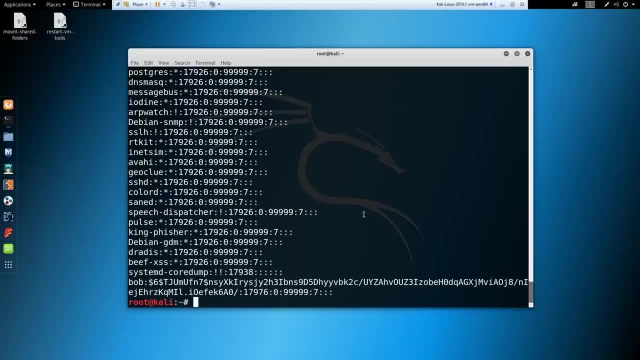 I have a video on how to crack these passwords, or the Linux passwords, with Hashcat. If you're interested in that, you're more than welcome to check out YouTube. It's one of the more recent videos that I have on there, And then we'll cover that and its importance more later down the road. 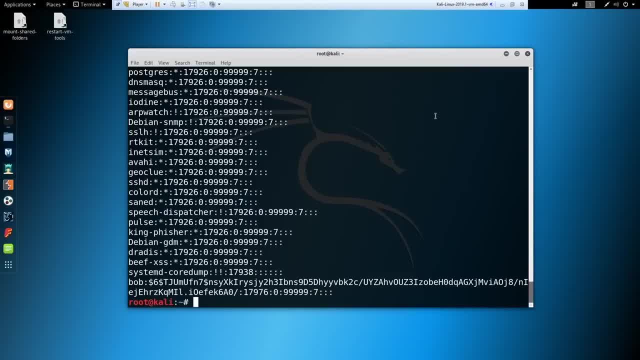 But just knowing that the Etsy password contains the users and the Etsy shadow file contains the hashes is what's most important. So, in terms of other users and permissions and things like that, a couple more important things we need to do- There is something called SU, which stands for switch user. 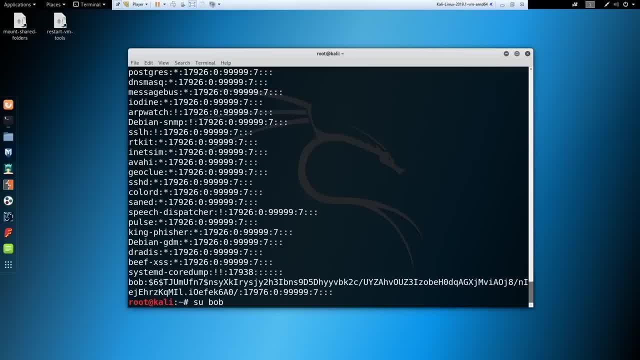 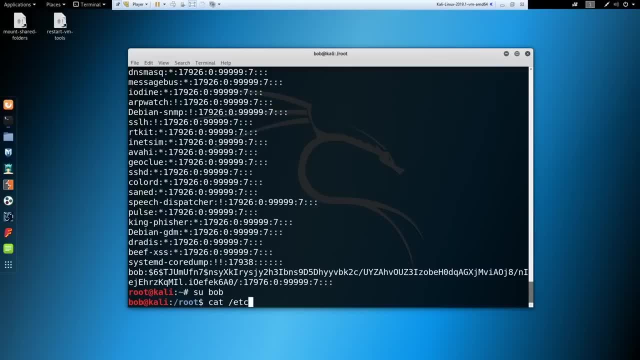 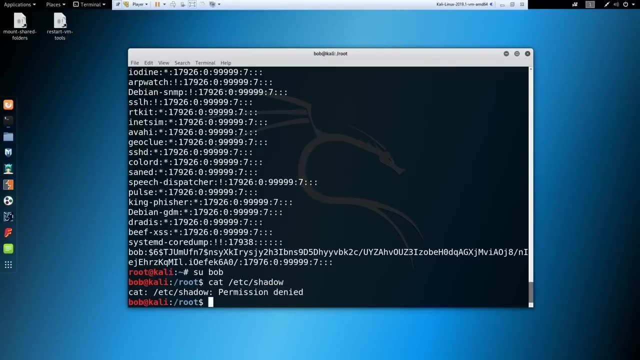 So if we say we want to switch user to Bob as root, we can just go ahead and do that. So now we're Bob. Now if we're Bob and we want to cat out that Etsy shadow file, we do not have permission to do that because we are not a sudoer. S-U-D-O-E-R. 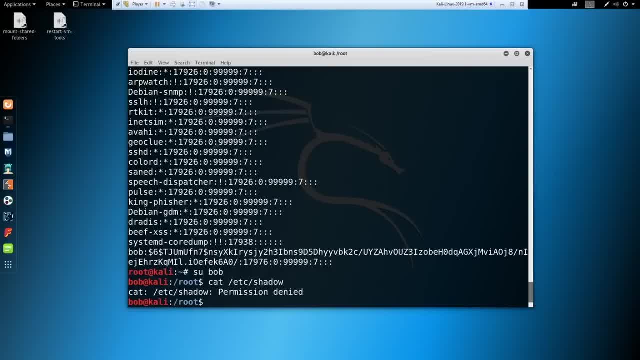 If we're not in the sudoer's file, we do not have permission to do that. If we tried, we could try to sudo cat Etsy shadow And then we type in Robert123, which is why I made the password. It says Bob is not in the sudoer's file. 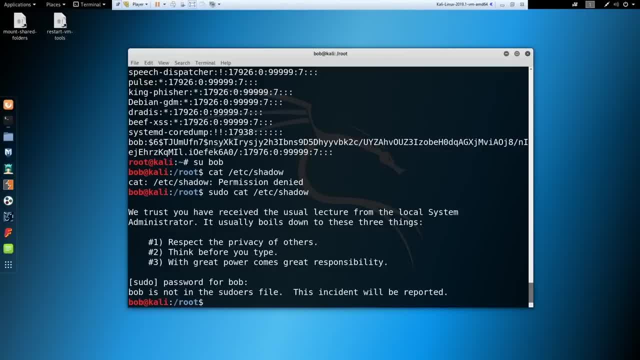 This incident will be reported. So basically, sudoers, is the permission for us. It's kind of like the permissions file. It allows us to have access or not to have access. Where does it get reported to? I don't know. That's a great question. 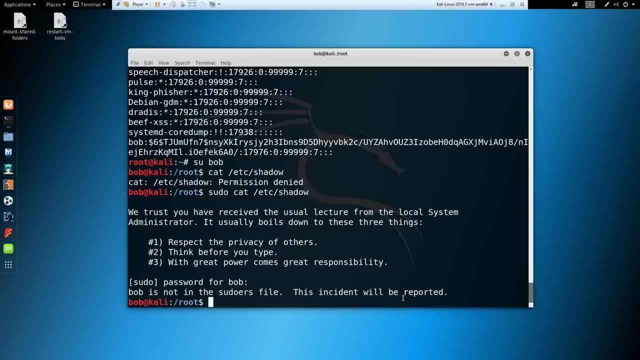 I have no idea. So if anybody knows that, I know some of you guys know a lot more Linux than I do, So please go ahead and tell me where that is, because I'd love to know. But anyway, so we can't do any permissions with him. 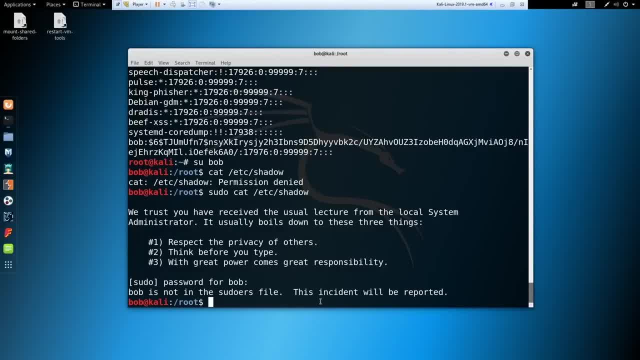 If we did, we'd use the command called sudo. So if you're a lower level user, you're not root, then you can't do that. If you're a lower level user, you're not root, then you would need to run sudo in front of your command in order to execute it at a higher level. 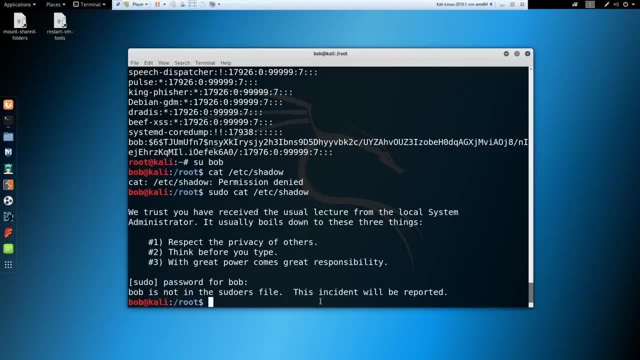 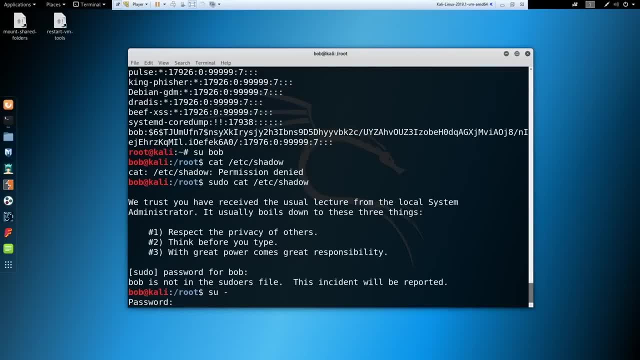 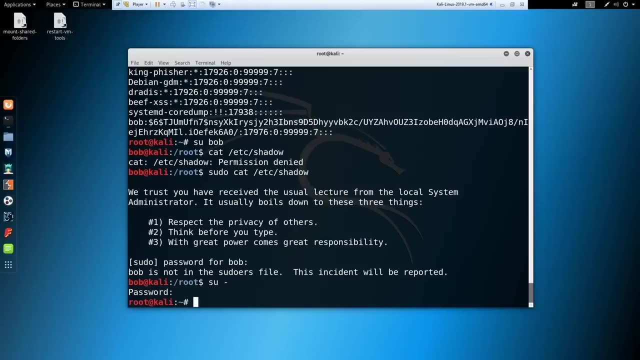 Did it get envar logs? We can look this up. I'm down, We've got extra time tonight So we can go. We're going to say switch user with a dash. See if this works. Okay, And we're root. 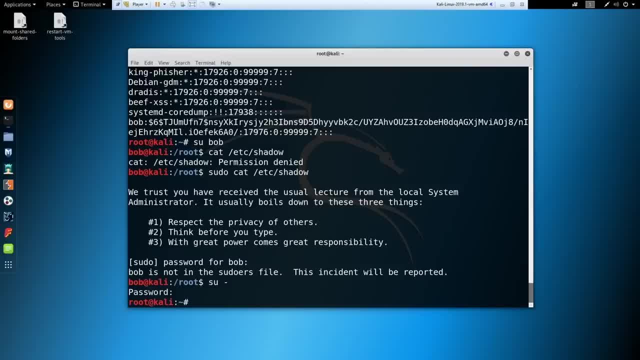 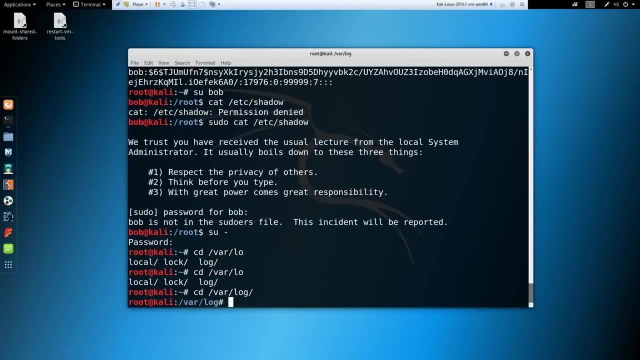 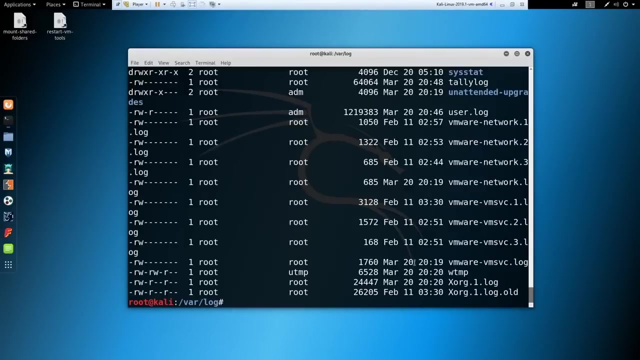 Let's put this back to root. You have to count out the var, the root file environment. What are you talking about? Var log, Can we CD? No, Yeah, Maybe What's the most recent people Hold on. 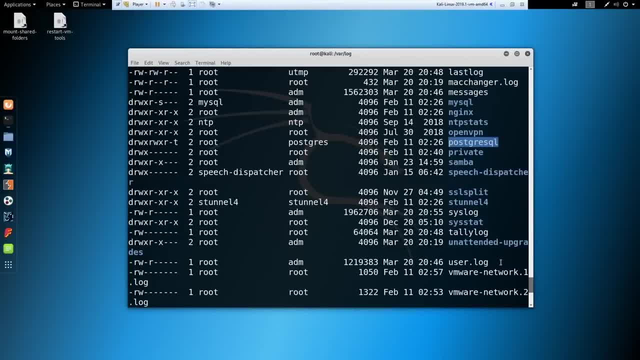 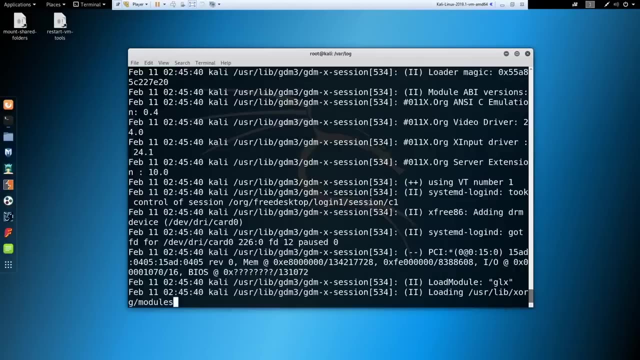 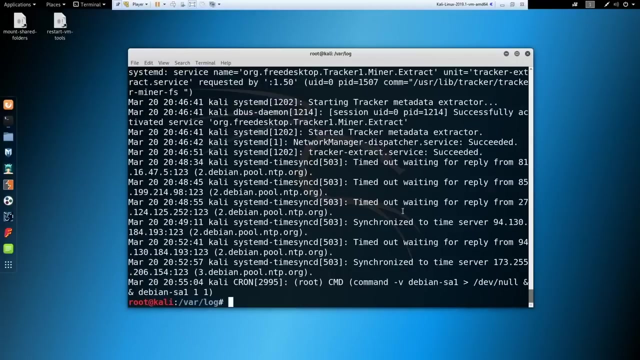 What are we looking for? Where's our? We've got March 20th Syslog, user log 2046.. That's not recent. 2055 is more recent. Yeah, Syslog. All right, Let's try something. 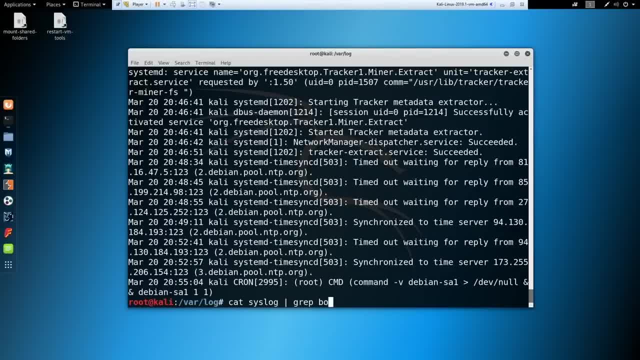 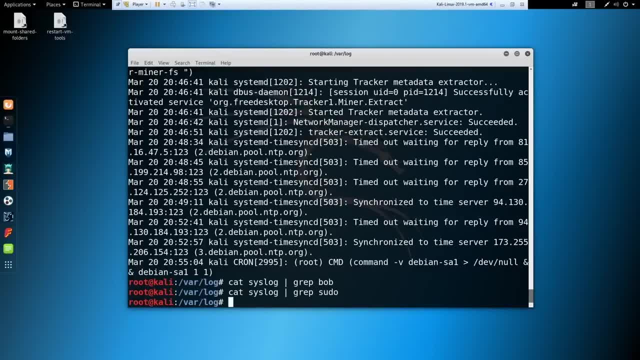 Let's try: grep Bob, No, grep Bob. Grep sudo- No, I just catted it, I don't. It's not. If you cd to var mail in LS, you get a file that says root Var log- auth dot log. 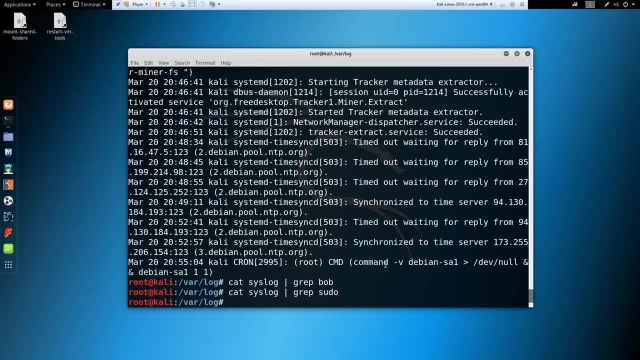 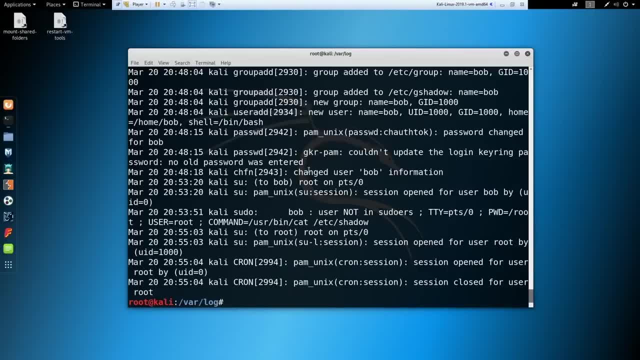 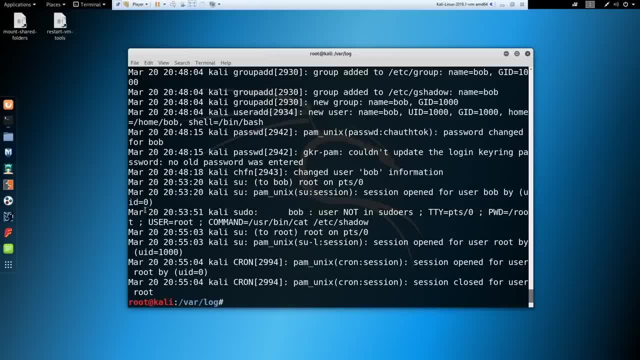 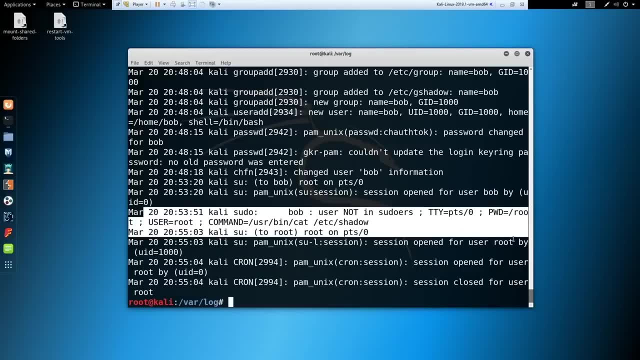 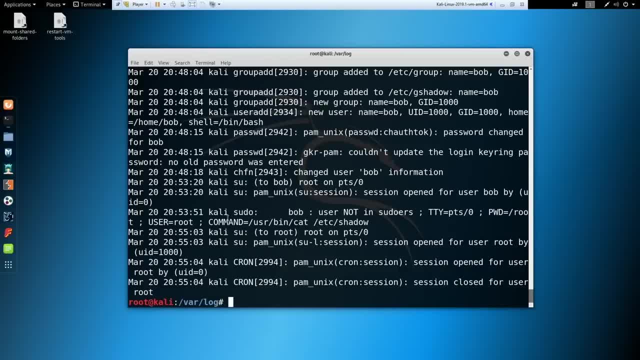 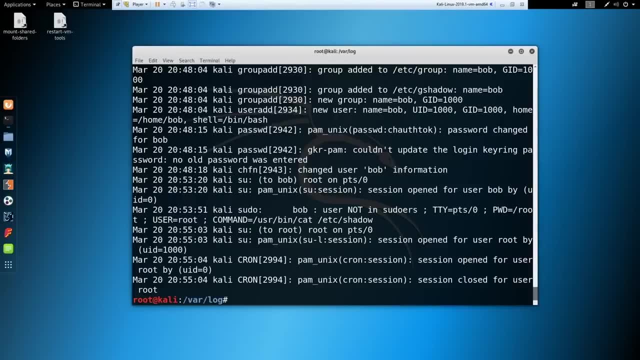 He's in trouble, Bob's in trouble. now, guys, Bob is in trouble. now You found it. Thanks, Davey. Davey's the best. All right, So that really covers it for the users and privileges. So next we're going to go into some common network commands. 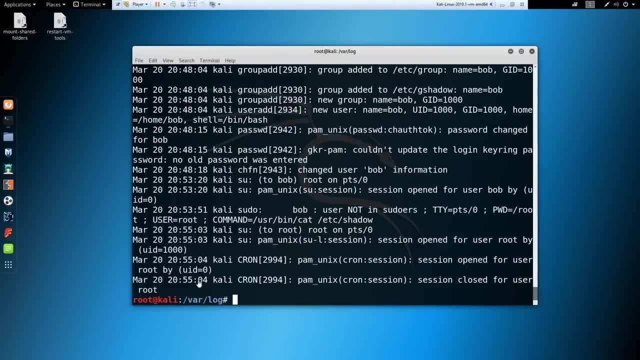 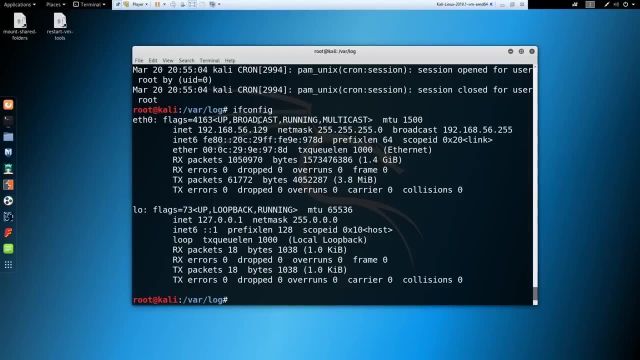 So let's go ahead and talk about those. So so the first network command that you should know, probably the most important command that you should know, ifconfig. okay, ifconfig is similar to IP config. if you are a Windows user, all this does is print out your information so you can see my IP v4 address here I net 6 is. 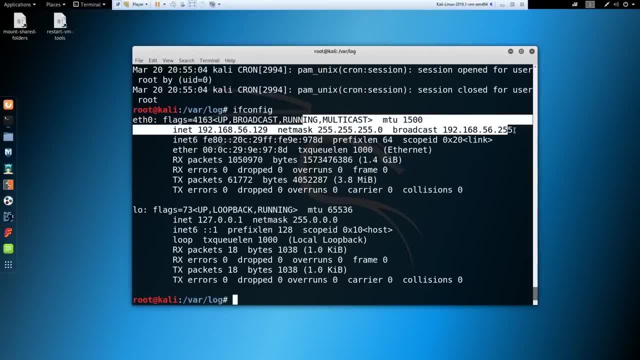 your IP v6 address. you've got your net mask, your broadcast, etc. if you are lacking on information when it comes to what a net mask is or what a broadcast address is, you may need to study up a little bit on your networking skills. this course, unfortunately, does not cover networking. oh yes, my IP is leaked, boys. 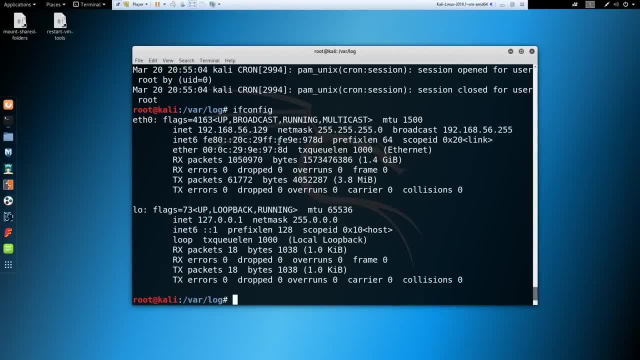 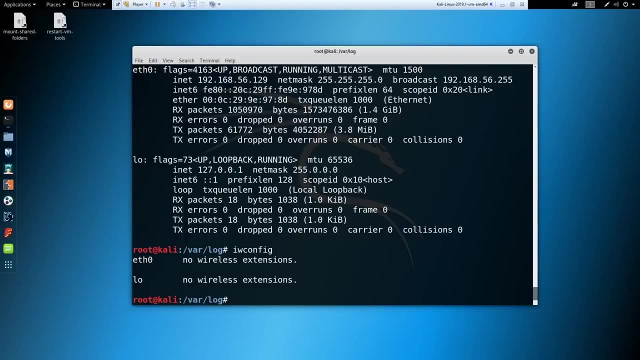 we're out there now. so this is for your, your Ethernet, your plugins, etc. the wireless version of your network is the wireless version of your network, and this is IW config, which I have no wireless adapter plugged in at the moment. if you're doing wireless hacking and you have a wireless adapter, then you 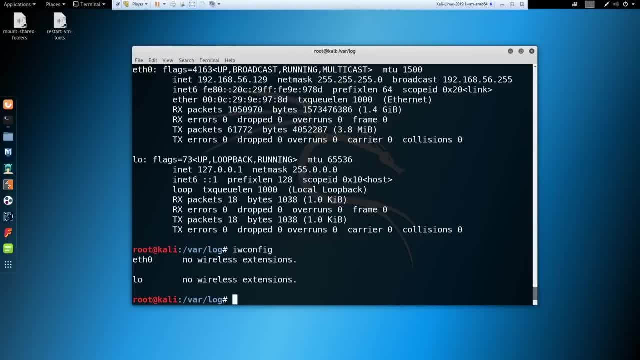 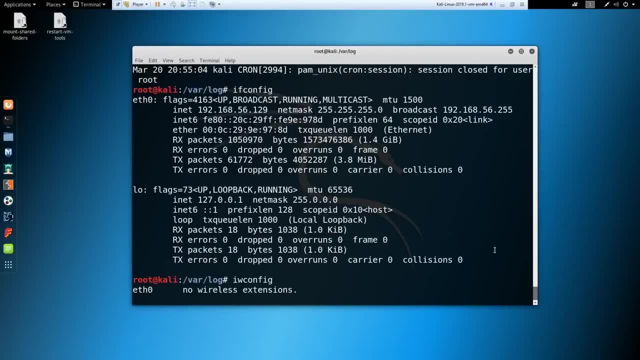 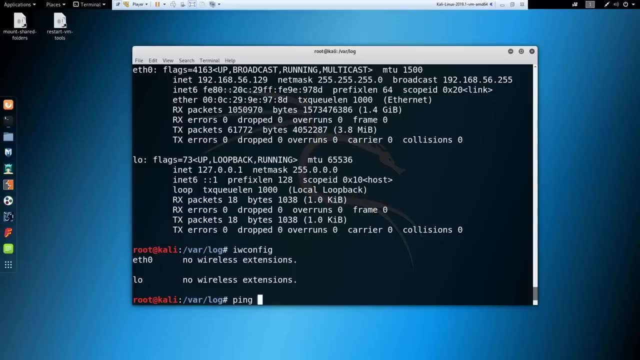 come into IW config and you can see that. okay, so from here, some things we need to know. one thing would be ping, right, so ping command, and we're going to talk about ping in depth later. so the first one is: IK45 is the greatest library for you to use when you're. 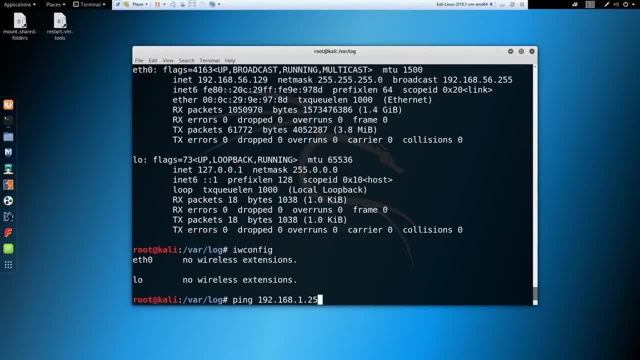 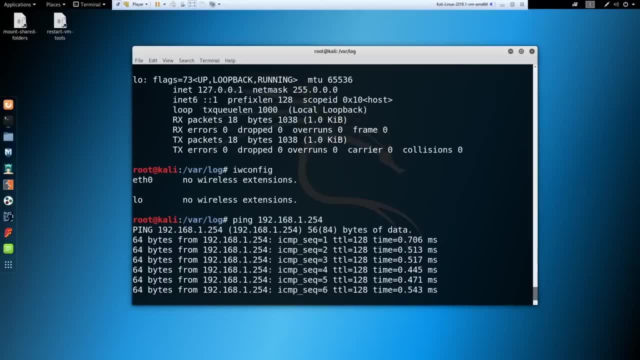 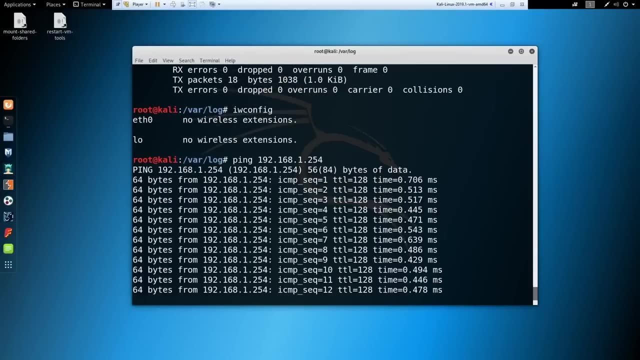 eating cuckoo in nossos house. um, if you ping, let's just ping something in our house. I don't even know what my. is it 2 5 4? yeah, 2 5, 4. ok. so you see, when I say ping, and I'm pinging something in my house here, it's just gonna ping. 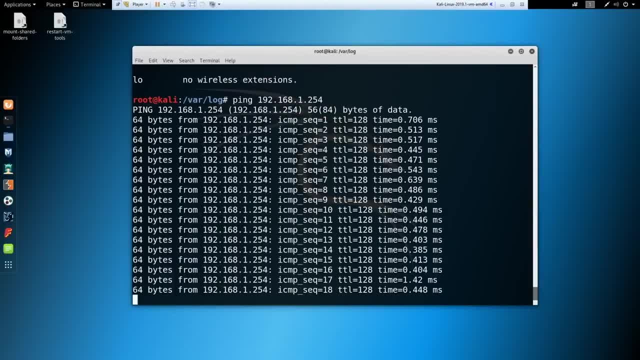 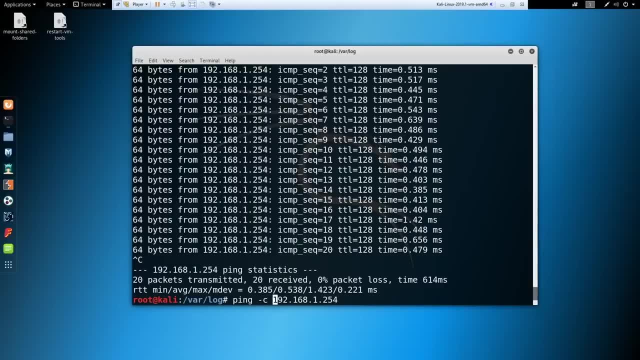 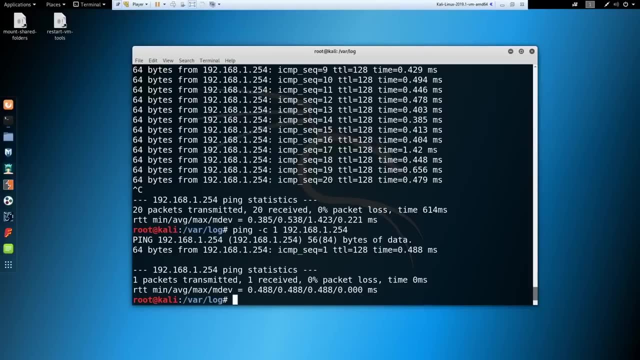 endlessly. I do have a room, bah. actually I love my room bah, but anyway. so one, two. if you want to ping it just one time, we can add a switch of C for count, say one, and then we'll just ping it once And again. we're going to talk about that in much more depth here. 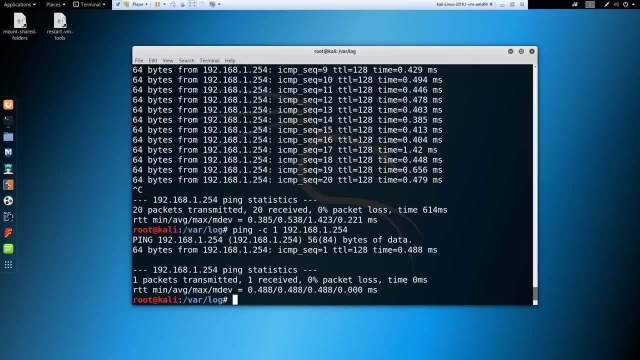 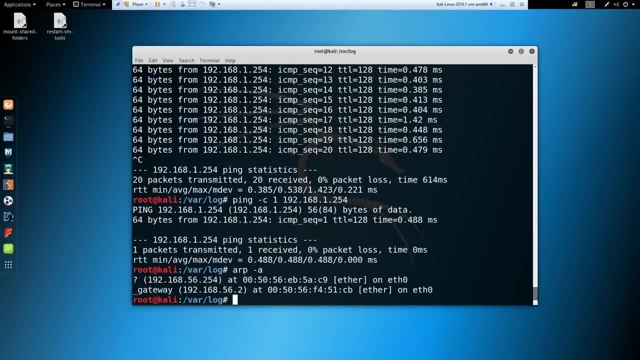 in a few minutes. Okay, another command that you guys should all know: arp-a. Okay, arp is going to be associating IP addresses with MAC addresses. Not a whole lot of information to go on here, but if you do come across it in a real world environment or even like a capture, 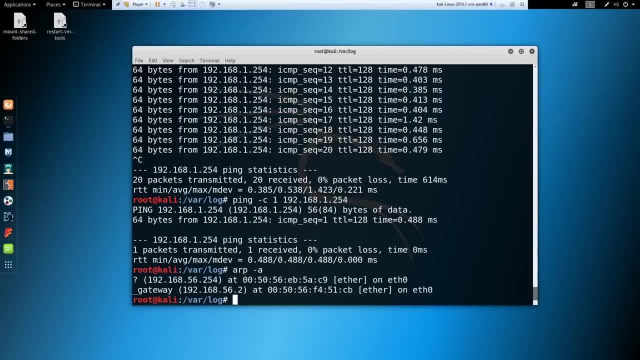 the flag network kind of environment. very useful to know Basically what's going on is. there is a broadcast address that's sent out and it says, hey, who has this IP address? And it says, hey, I do, Here's my MAC address. right, They associate the MAC address with an. 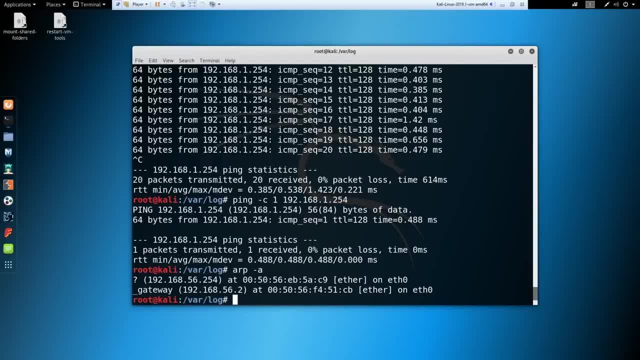 IP address. So this is really good if you're looking for, like, dual home networks or if you're looking for a machine interaction, Interacting with another machine that you weren't aware of. ARP is really, really awesome. So another command that is important is netstat, And I like dash A-N-O. 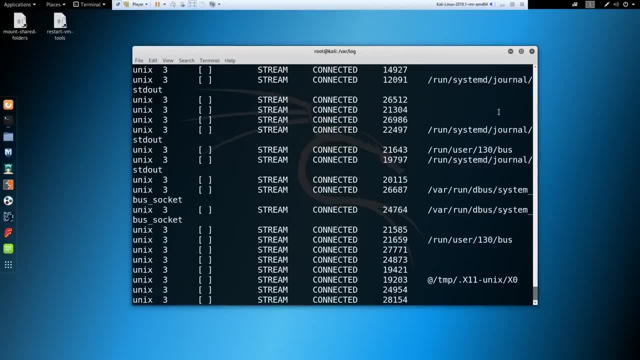 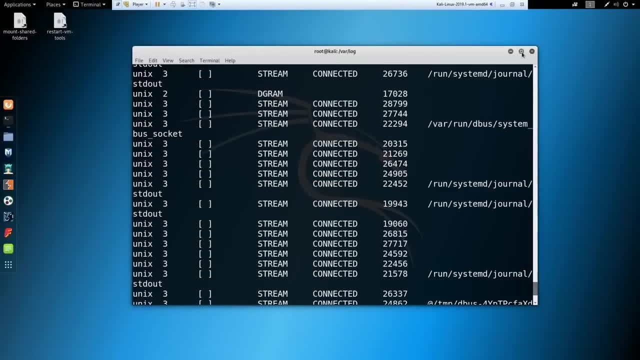 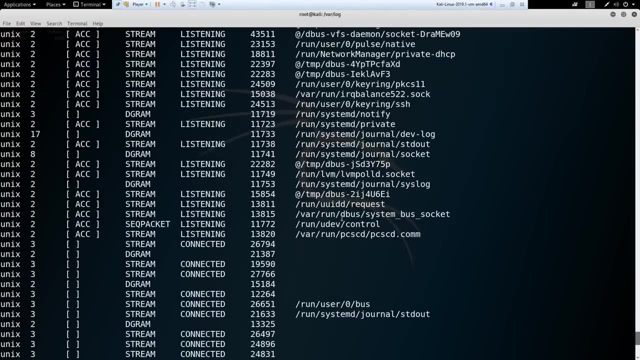 So netstat shows you all the ports that are open and it shows you what's connected to those ports. It's, I think, prettier when it's on Windows, but you can come through here and you can look at the different types of connections that are running on. 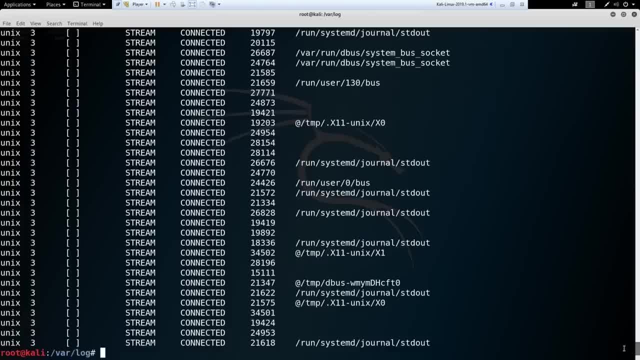 Very useful command, especially when it comes to again seeing what ports the machine has open, what it's talking out to. This is a good way to become paranoid. So if you go onto your computer the first time, you run netstat and you say, oh my God, what are all these ports that are open? 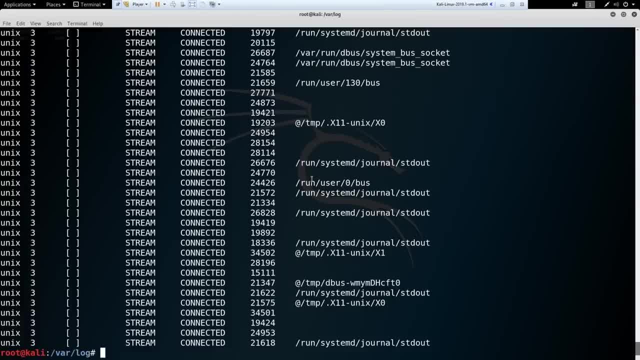 I don't know those ports. You spend a night of paranoia the first time you learn about netstat- At least I did And I know some other people that did too. But when it comes to machines, like say, we're on a Windows machine and we run netstat and it's got. 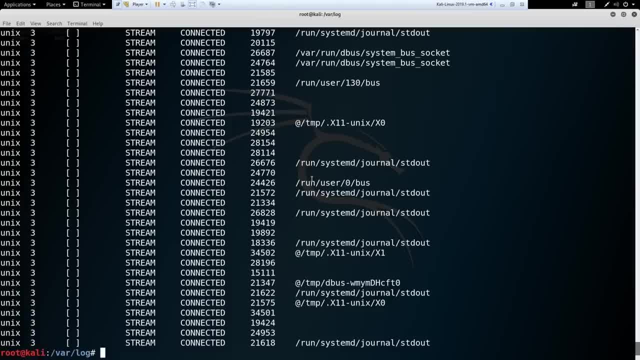 open ports. we really want to know what we're talking to, right. If that machine's talking to something else over a port or it's got something open that maybe we missed in a scan, we want to know about that And we want to know what ports that maybe it can talk out on. 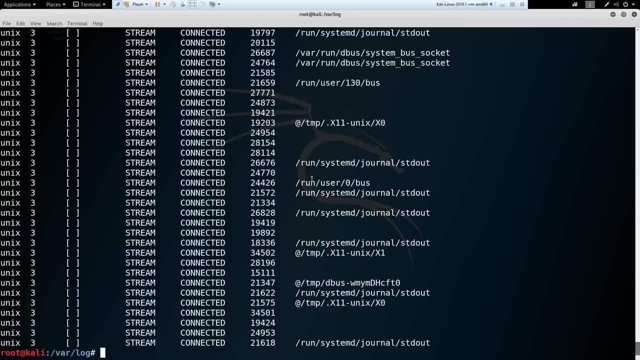 et cetera. So there are some commands we'll learn later as we go to kind of find out this information, But for now just know that netstat exists. Okay, so the next command is the route command. So we just say route. This is our routing table. 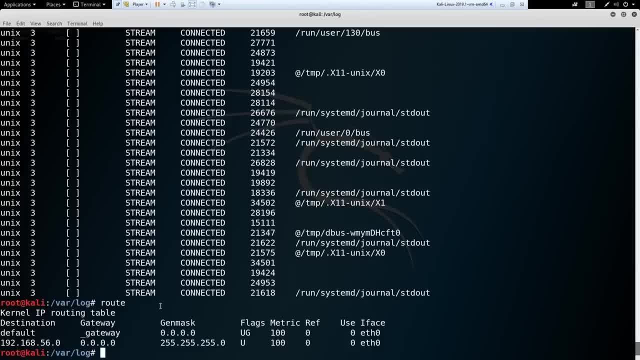 So you can see that again, not very interesting. It's more interesting when you actually have a network going on. But this is something to look at as well because, like I said earlier, if we're talking dual home network, say that we're sitting on 192.168.56.1, but we also have a 192.168.56.1. 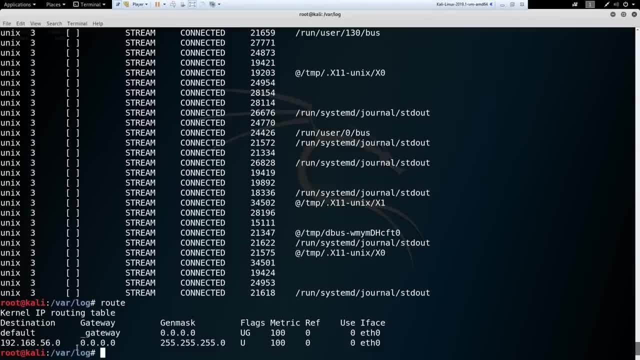 or something like that. right, And this gateway of all zeros, okay, we're out there, And then it shows us the Net Mask or the Gen Mask, And then it has metrics and stuff. And again, if you don't know networking, you might want to look some of this up and kind of look into it. 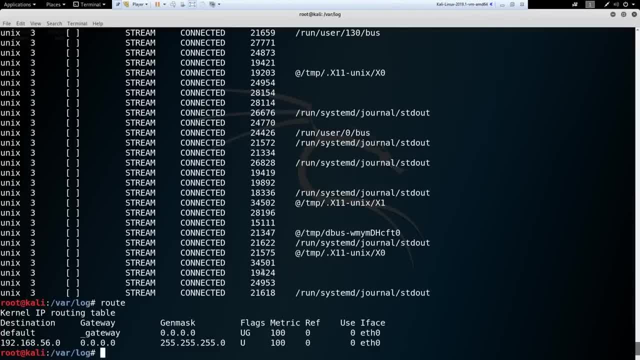 and see what it's all about. But again, it's very important to look at from a pen testing perspective to see what that machine's talking out to. How long has it been up to? I've been hacked before. I've been hacked several times. I'm always working on the next step. 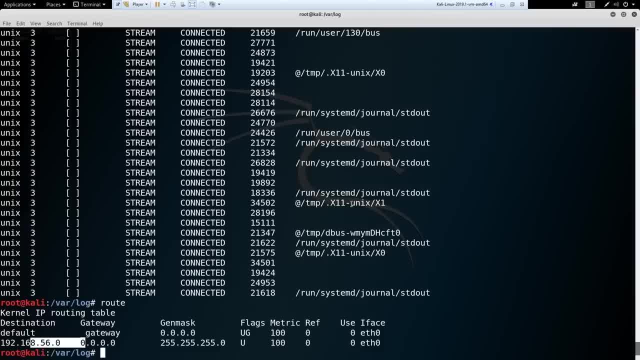 It's like I'm going to go in and come back and click it. I've been hacked for a while. I've been hacked for a while. I'm always working on the next step. I've been hacked before. I don't know if I should admit that. 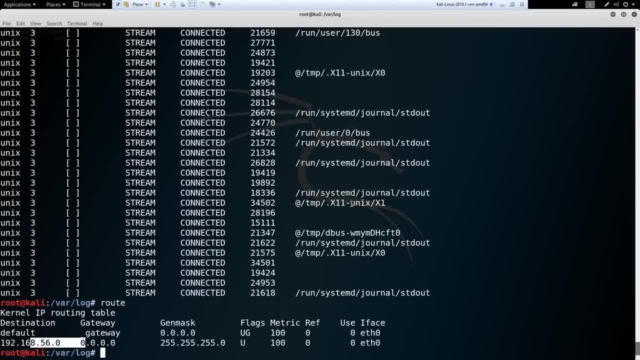 Like back in the AOL days when they would send out that hey, your friend would say, hey, you know whatever that was called. they say open this file, And then they would start opening your CD-ROM drive or whatever it was you know. 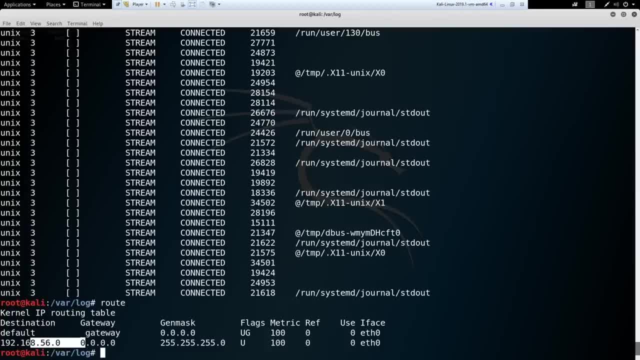 they would like, they can control your mouse. There was a name for that stupid malware, But that was a good one. I also got malware from. I never got it from LimeWare, but Kazaa, Kazaa was it man. 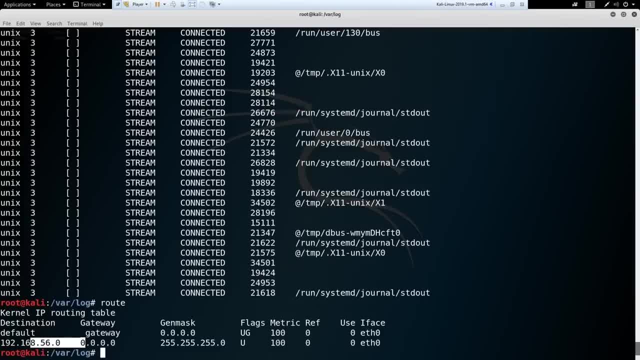 Also my young innocent days. I was trying to download a music video and definitely did not get a music video. So you know, All right guys. So that's really it for common network commands. So we're gonna go into viewing. 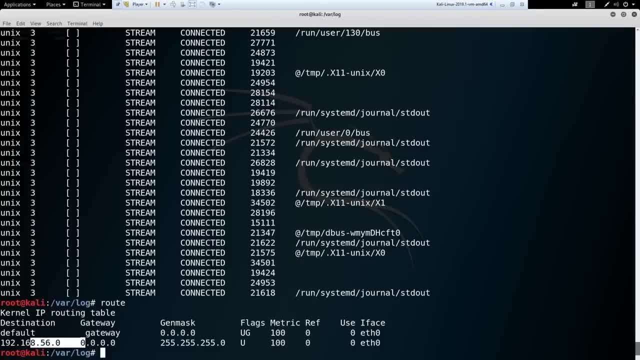 creating and editing files. After that, we're gonna do a little bit of installing and updating. We'll talk about services, which will be really quick, And then we're gonna get into scripting, which should be pretty fun. Yeah, I actually remember the music video. 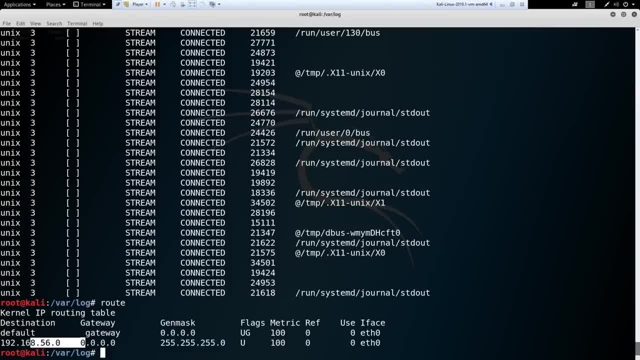 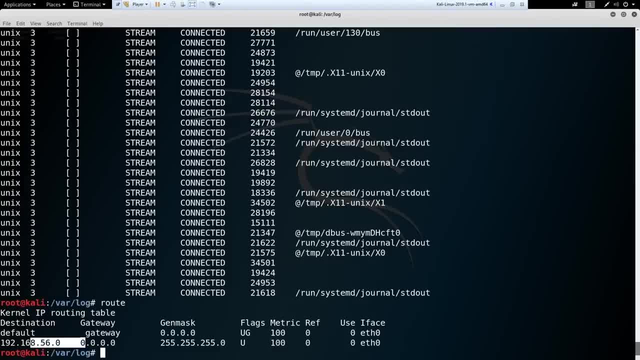 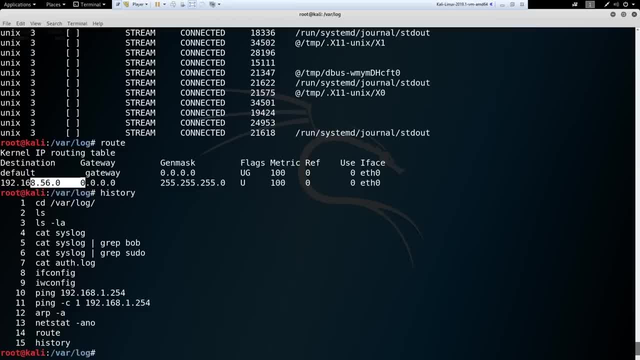 Okay and you can see like all the history of the commands I've typed recently. but where this becomes useful is if you're trying to find a command like there's so many tools and so many things that you run as a pen tester. 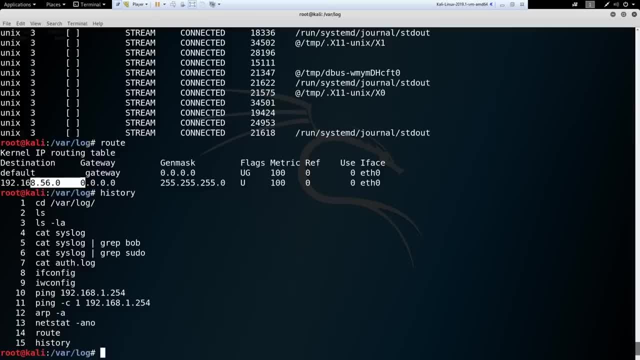 that you kind of forget all the syntax that you run over time, right? So for me, if I want to run something like say, I forgot you know how to run ping, I would say history grep ping, And then I would see all the times. 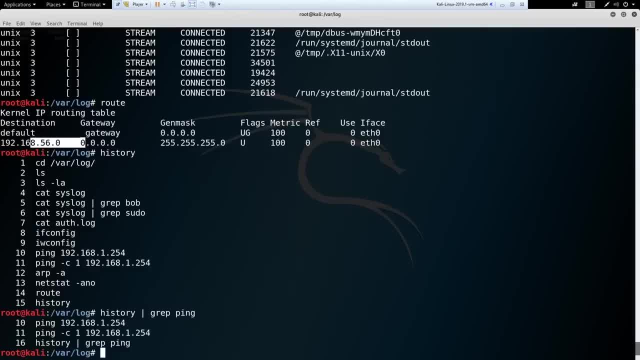 I've ran that history command or the ping command and find out exactly what I need to run. So it works out really well, cause I can never remember all stupid switches and everything that goes with these tools. So, okay, let's talk about viewing. 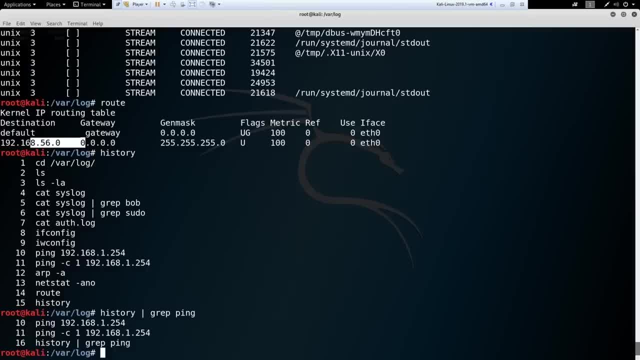 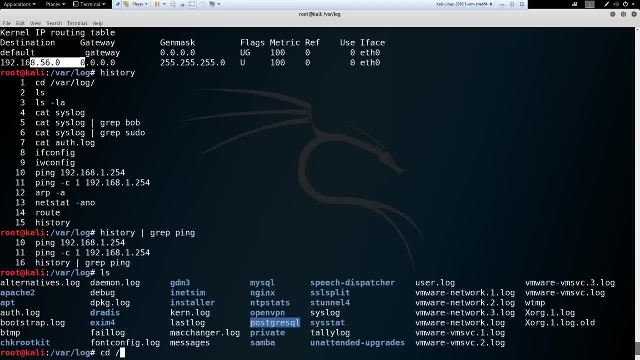 creating and editing files really quick. So if we say LS, let's see what we got here, Oh, we're in bar log, Let's go back. Let's get to root downloads. Another way to do this is you could just a tilde. 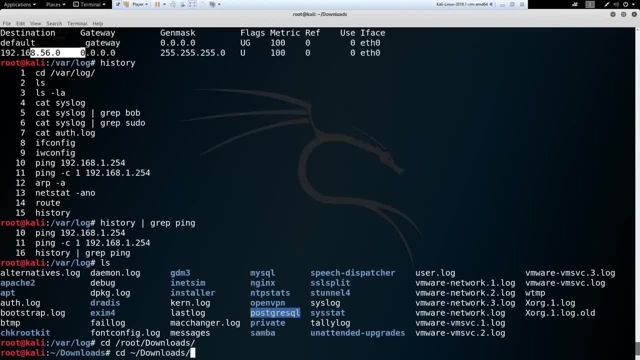 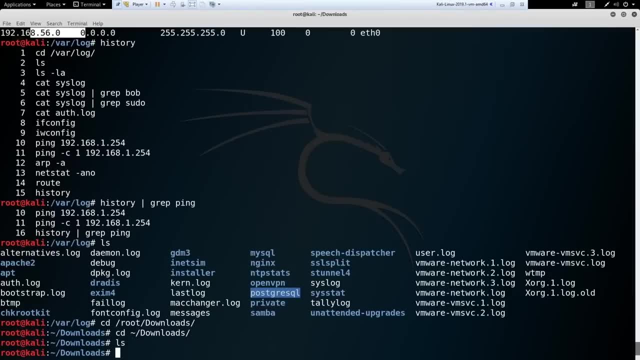 like that little. you could do CD, a tilde and then downloads if you wanted Cool little trick, If you guys like cool little tricks, So LS, nothing in downloads. Okay, so we're going to make some files here. So you saw one way to make a file earlier. 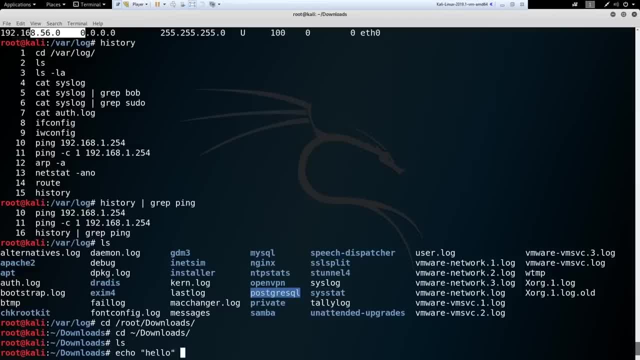 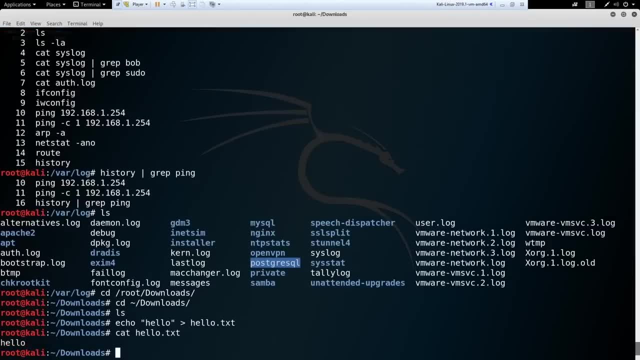 I just echoed hello And then we put that with this caret in here to hellotxt And we could say cat hellotxt and it'll say hello. Now we could also say: okay, let's say hello again into hellotxt And let's just leave it like this. 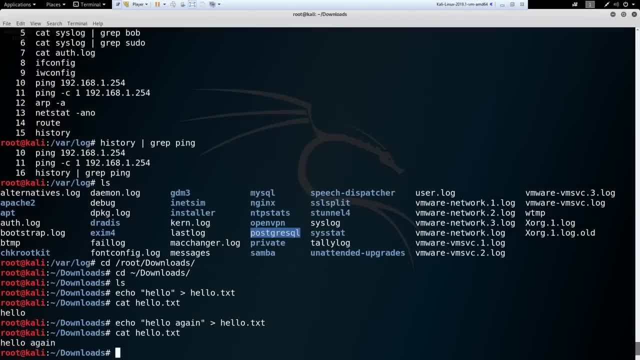 Hit enter and let's say: cat hellotxt. Okay, well, we just overwrote the file. So be careful when you're using these carets here, because you want to make sure that if you want to write an additional line to a file, that you use a second one. 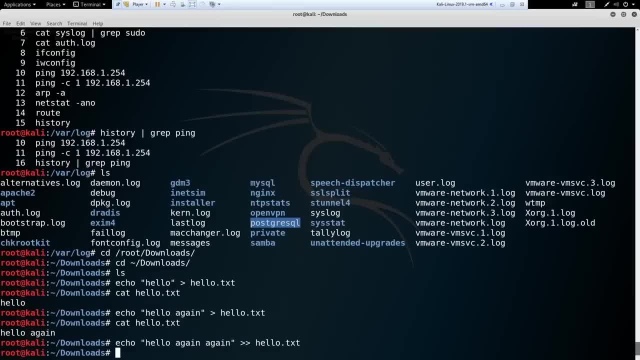 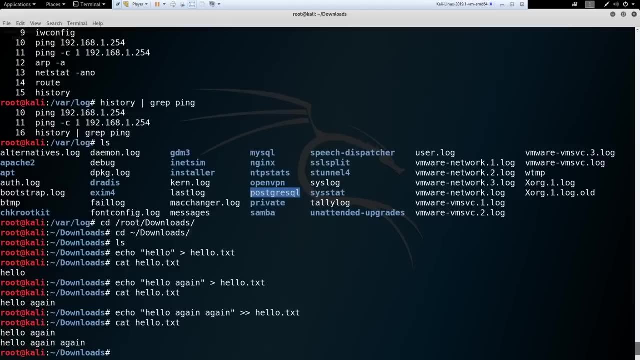 like this: say hello again again. look at you special little students. Cheshire and Redfinite Allie, you guys are going to the advanced class. You're in honors now. Okay, so now we've appended it, So we've got hello again, and hello again again. 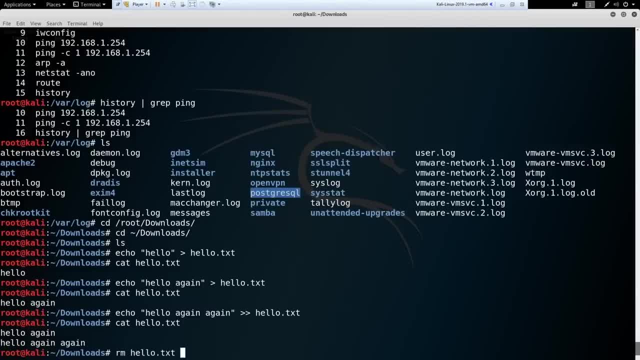 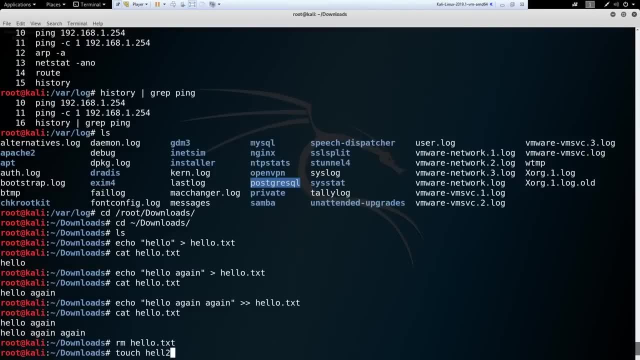 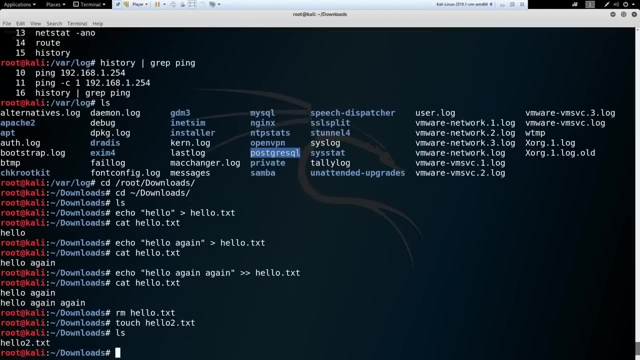 So we can remove this file. And another way we can make a file is we could say: touch hellotxt. I'll make a hello too. just for proof of concept: LS, Hello, twotxt is there. We could say: nano, hello threetxt. 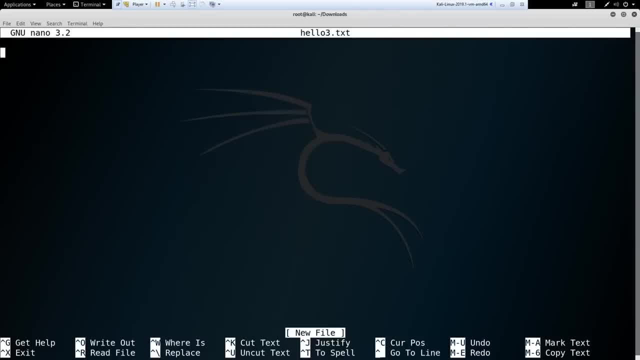 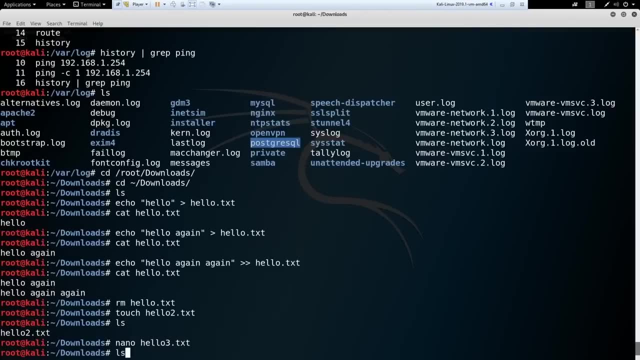 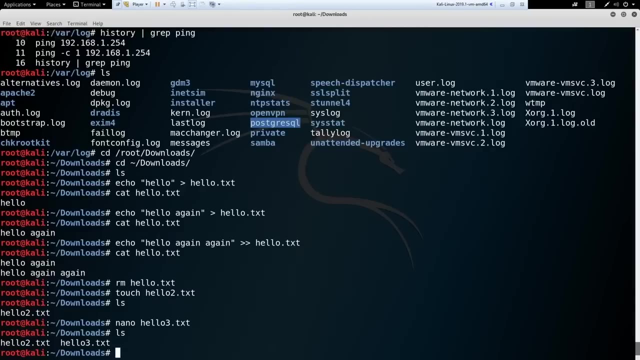 Can't type guys, And then we could say hello and hit control X in here, Say Y for saving and enter ULS. Hello three is there as well. No vim, no vi, none of that, None of that. Nano is great. 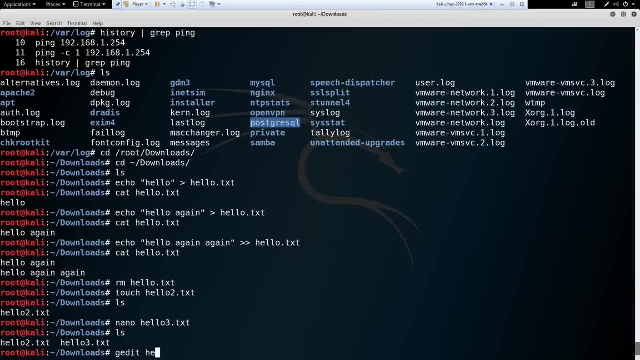 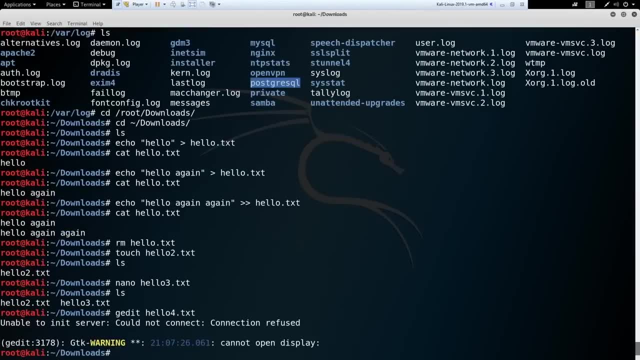 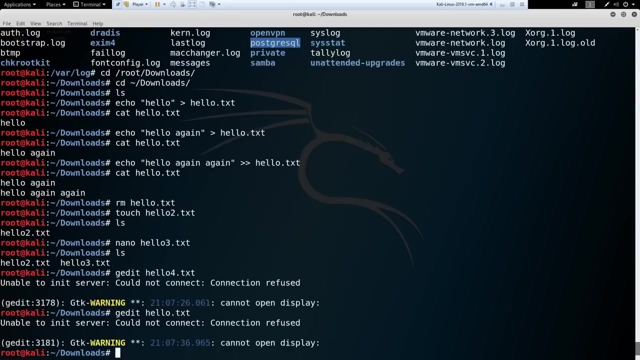 And lastly, if you're a gooey guy, hello fourtxt. I'm using gedit, No gedit. what is going on, guys? Is this new? Is this new? I've never seen this in my life. Not installed. 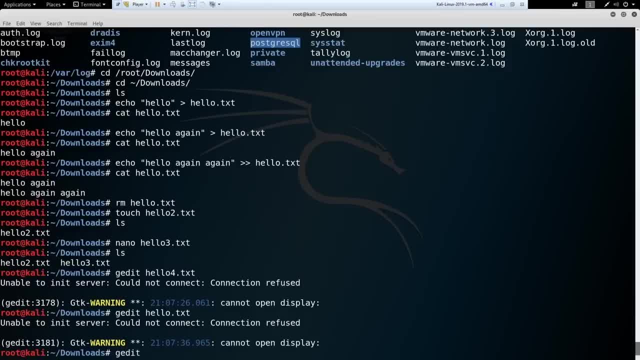 It's installed. Look at it. Hello, tab gedit works. There's no two Ds. It was taken out. What are they doing to my like? okay? Well, we'll get to app. get here in a second. 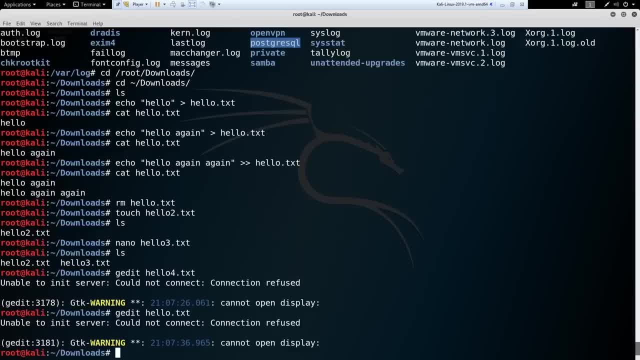 That's one of the next ones. Okay, no gedit, We'll talk about gedit. Let's get right into installing tools and updates. So let's see if we can app get install gedit. See if that works. No, I don't want to download. 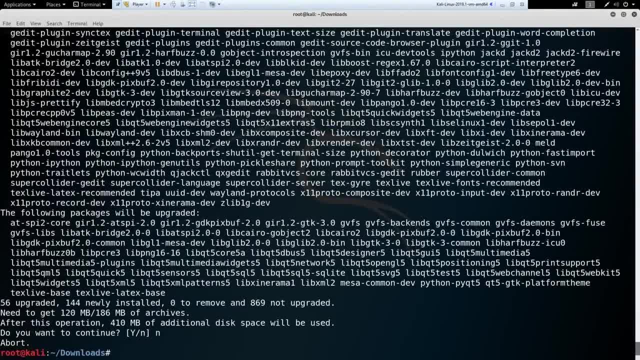 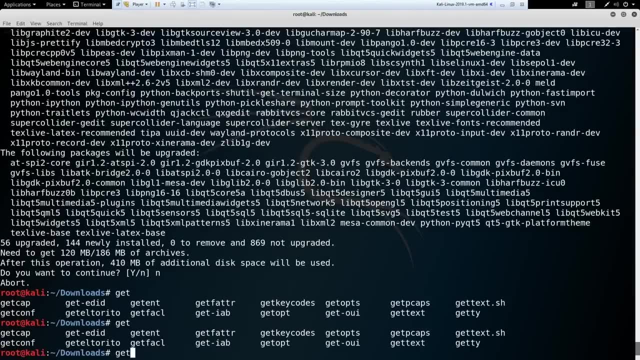 410.. It's not worth it, guys, Not worth it. No, apt, Is it just get? now, What are you talking about? Is it just get? I don't know all these App: get install windows, Just apt. Why are they changing everything on me? 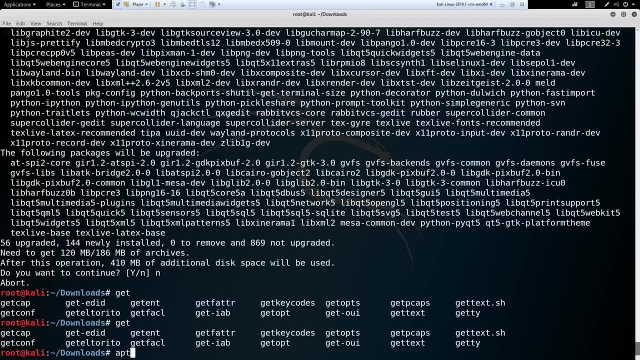 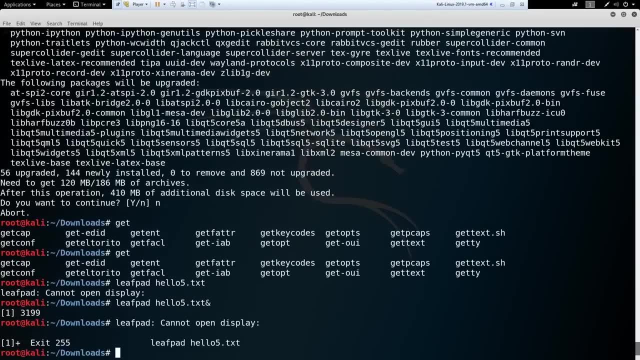 Anyway, you have graphical editing choices: Leaf pad. Do we have leaf pad? Can we just call leaf pad? Hello, five dot text Cannot open. It hates us, Cannot open, Still hates us, guys. I have to ask politely: 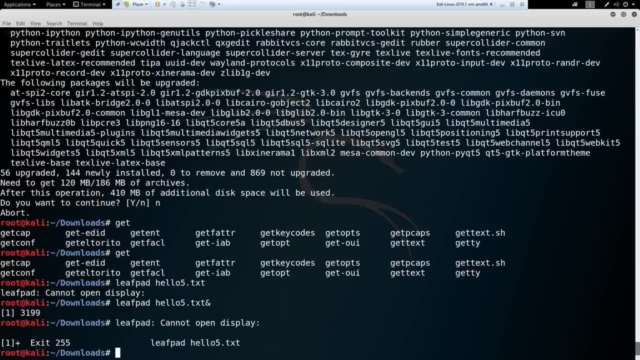 All right, we'll skip it. Just know that gedit works. So anyway, all right, we're going to do this without running apt-get, apparently. So if you want to update your machine, if you want to do updates, you could say apt update and apt upgrade. 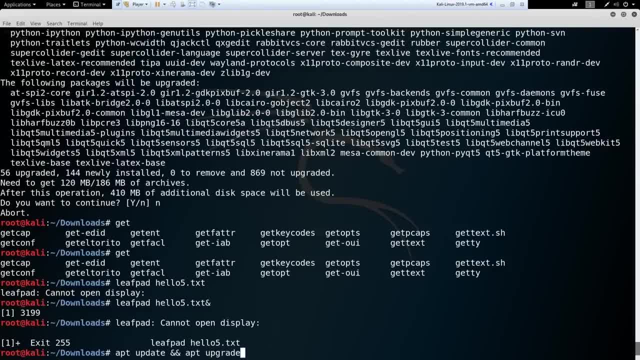 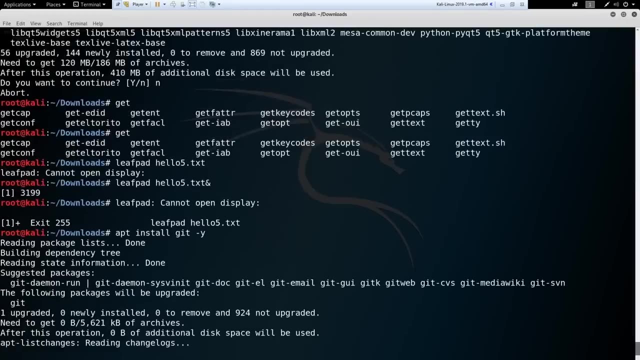 You don't want to do this right now because it'll take forever, But this is a good idea. Apparently, I need to do it because my shit's broken, But I do want to show you how to install some tools. So the first tool I want to install is apt, install get, and we're going to say a dash y just to say yes on this. 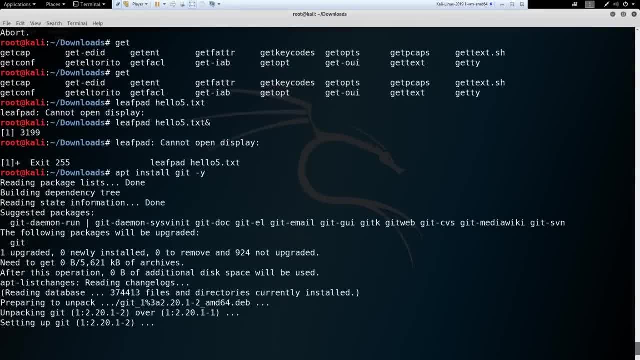 Basically, it just accepts the install automatically and starts installing it for you. Get is a useful tool that we'll be using quite a bit, I'm sure, throughout this course, And I'm going to show you an important install that we're going to do with get tonight. 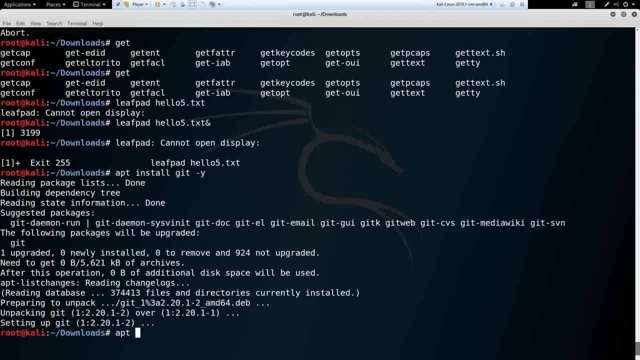 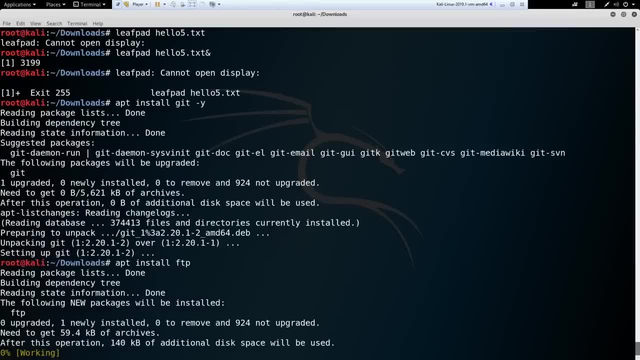 So we've got get installed. We're also going to install FTP, because apparently by default FTP no longer comes with this machine either. So I don't know what they're doing, but they're ruining everything that I ever knew, And apparently we're not able to connect to archivelinux. 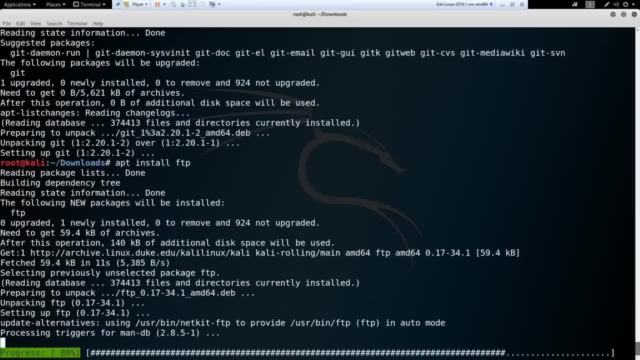 Oh no, there we are Okay, So make sure you get FTP installed as well. I'm trying to run the same commands and the same everything Because you guys, from the beginning I don't want to use my personal one, because I want to make sure that any issues that you guys encounter I also encounter. 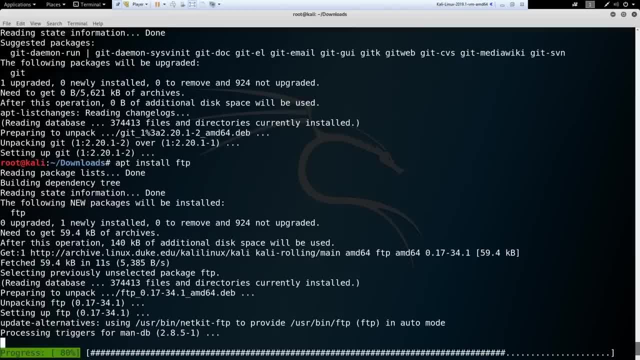 Yeah, maybe we're going to switch to Parrot. Maybe we'll do this lesson over again next week. We'll do it in Parrot, Okay, So while we're waiting on this, let's go ahead and open up a Firefox session. 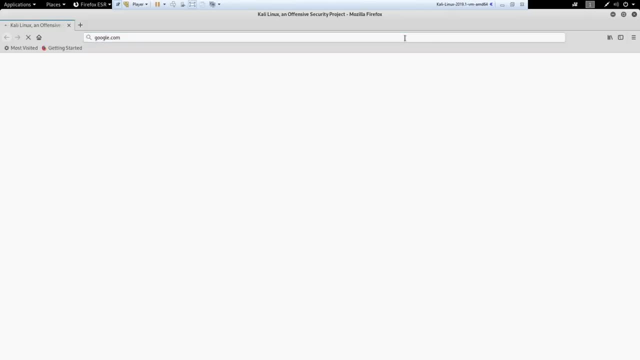 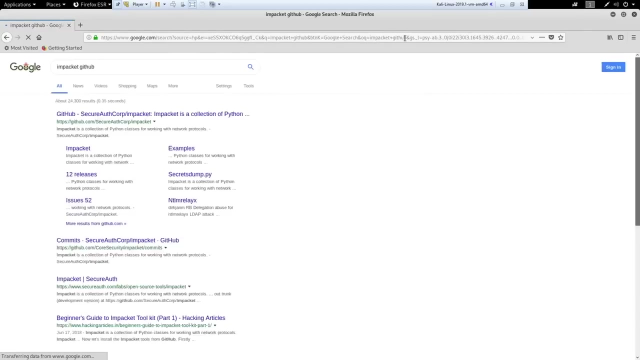 And we'll go to Google. What we're looking for is we're going to be looking for something called mPacket. So we say mPacket And I'm just going to say GitHub- I don't ever remember. Okay, So this secure auth corp mPacket right here. we're going to want to grab this. 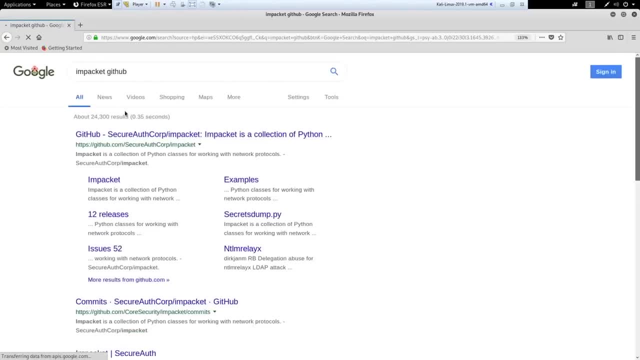 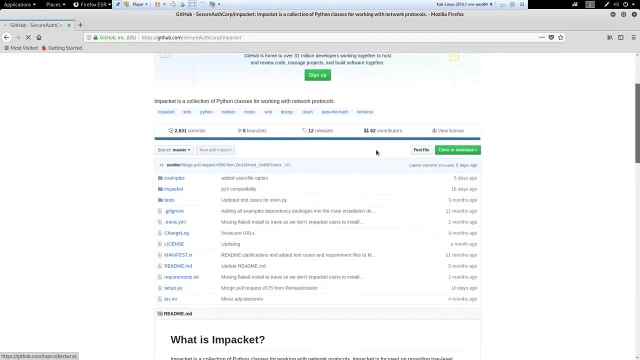 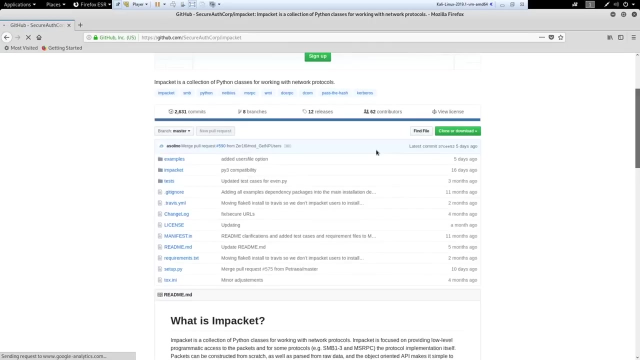 Let me control plus. Okay, so we click in here and this mPacket tool is something we're going to use quite a bit when it comes to internal penetration testing. You may have seen me use it before- last week we did when we did active- or two weeks ago when we did active, we used mPacket quite a bit. 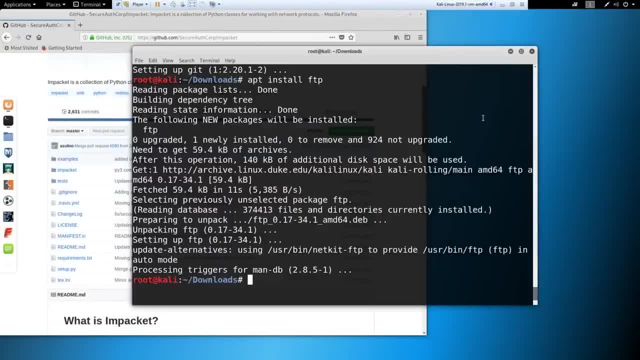 So what we're going to do is, by default, the Kali version of mPacket is broke, Unless it's fixed in this recent version. Okay, Recent update? I don't think it is. We're going to go ahead and fix it ourselves. 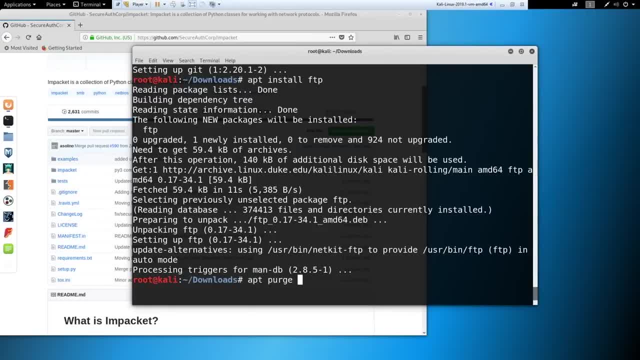 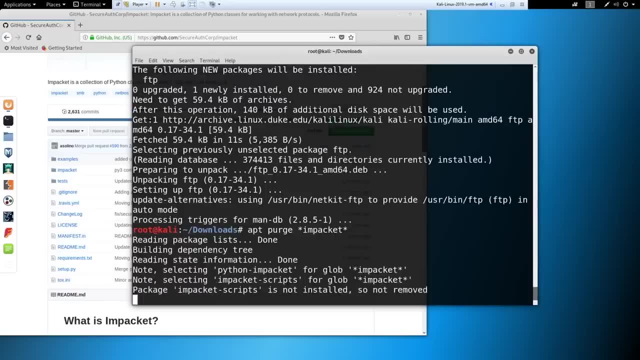 So what we're going to do is we're going to say apt purge, So we're going to get rid of- and I just put a star around it. I want to get rid of everything that has to do with mPacket. Let's just get rid of this program. 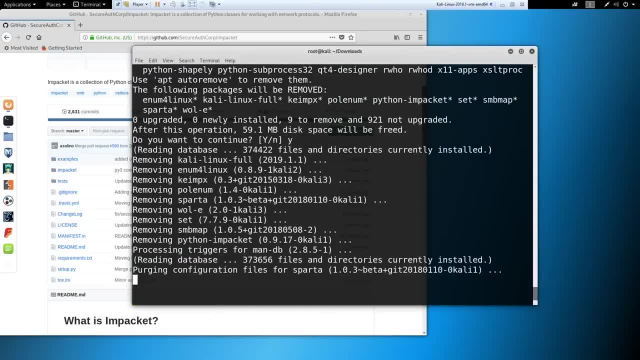 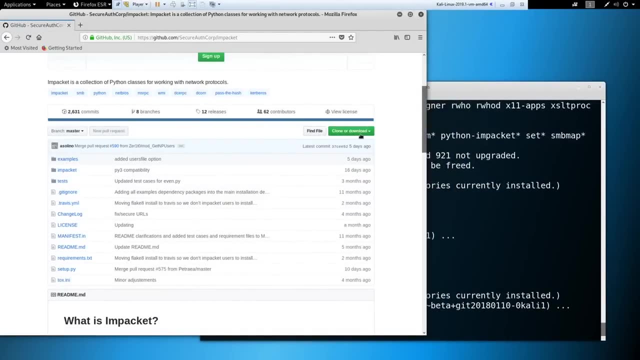 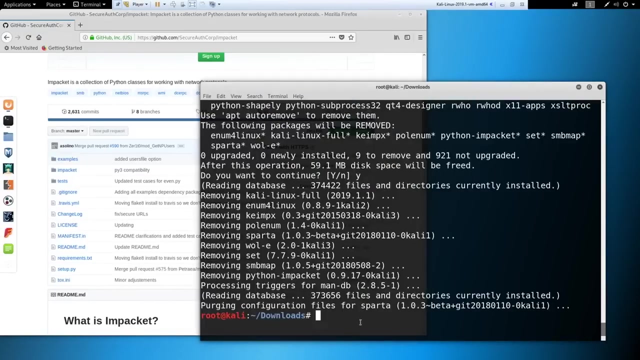 We'll install it ourselves. So while that's purging, what we're going to do is we're going to actually Copy this address in here. So if you go to this, clone or download And you just copy this link, Okay. 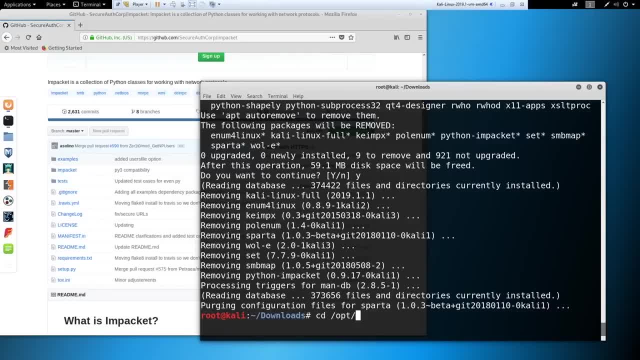 So what I'm going to do is I'm going to CD. I like to put this into opt. I like all of my programs in the opt folder. So CD, slash, opt. And then I'm going to say: get clone And I'm going to paste this into here. 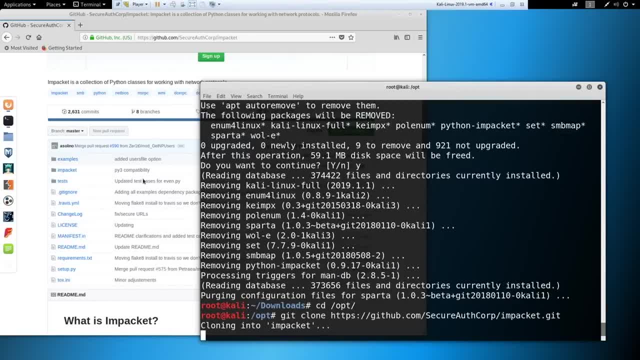 And it'll clone this file, all of this from the web, And we should have a nice little mPacket here in a second. I don't know what's going on. Everything's going slow, Okay, So let's see CD mPacket. 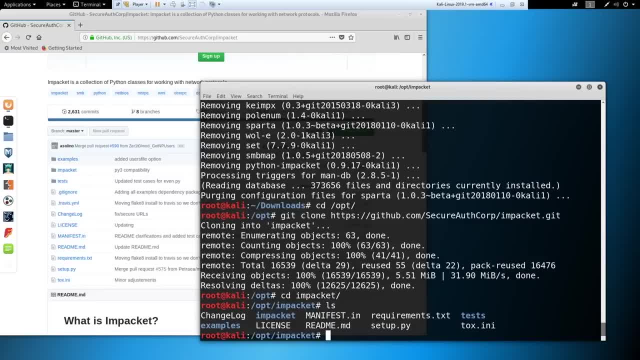 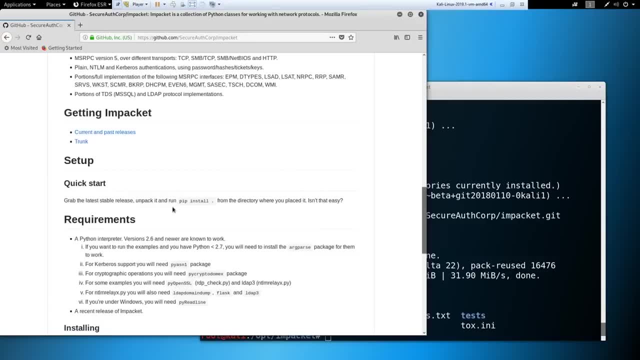 Okay, LS. So what we need to do is we need to read this and say, okay, What's going on. What's going on, What's going on. What do we do? How do we install it? If you come through this install guide, it says you run pip install period from the directory. 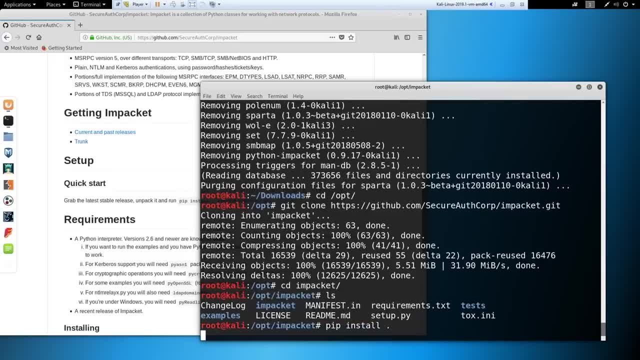 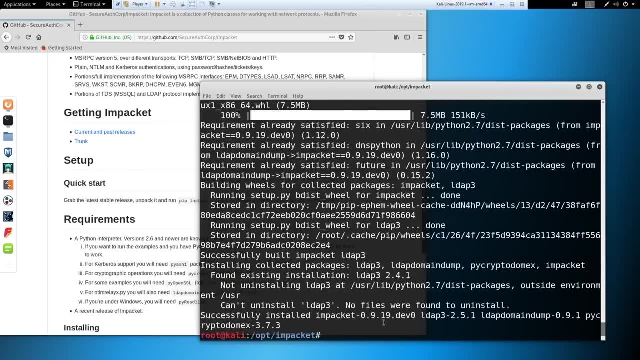 And you say, okay, pip install period And that'll run the installer for mPacket. It's as simple as that. except we don't have LDAP3. So we'll have to work on finding that as well. So no files were found to uninstall. 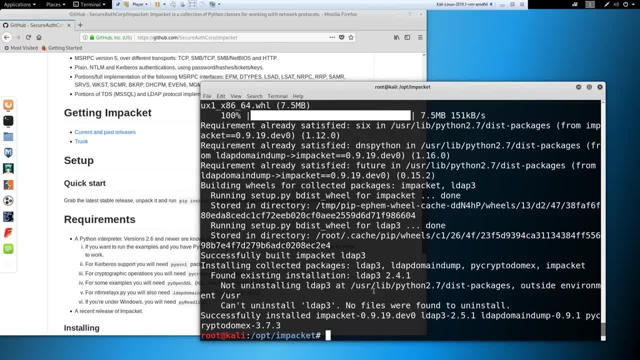 Oh, we're not uninstalling LDAP3 because we already have it. So that's good. I think we're good. So that is how you kind of install or uninstall applications. So you saw the purge, You saw the install And then you saw using Git. 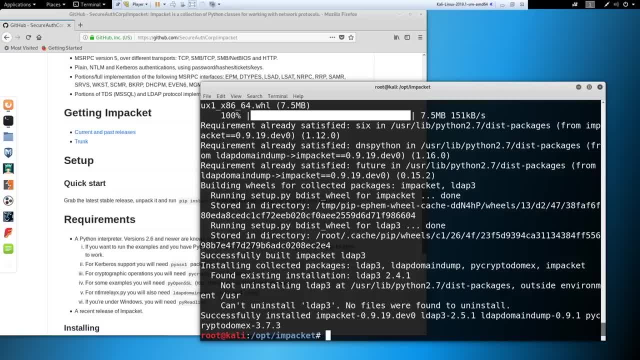 So Git's going to be very important. Okay, So when we talk about controlling- Next controlling Kali services- I'm going to teach you how to turn on and turn off services. You're going to make them feel really good about themselves. 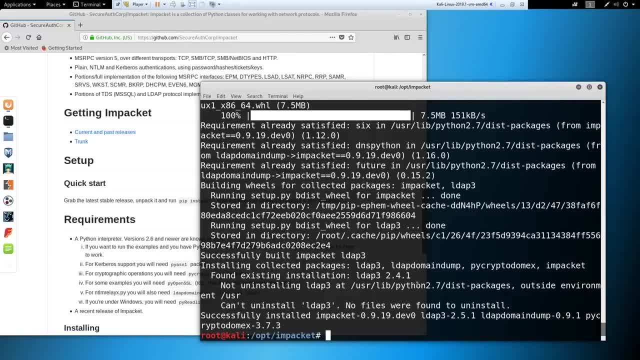 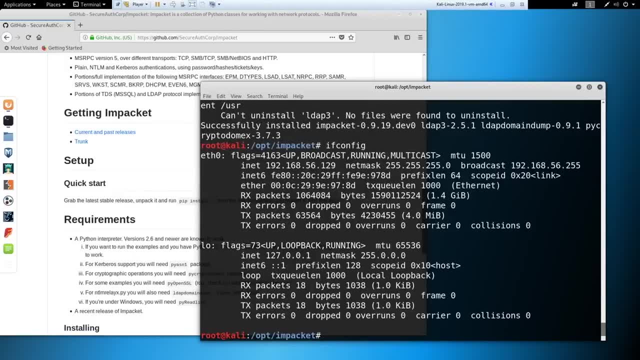 So what we're going to do here is: let's go ahead and do an ifconfig, Let's pull our IP address. All right, Kev, You're ahead of the class Kev. So we got our INET address, That's 192.168.56.129.. 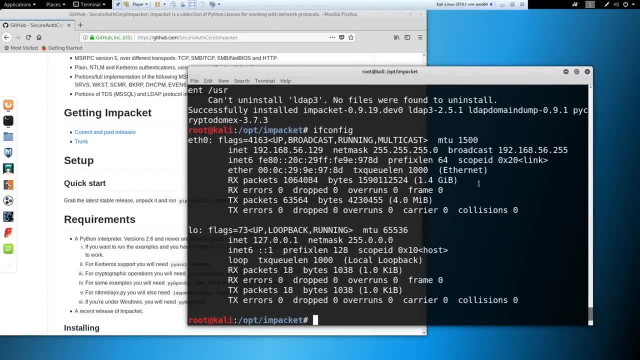 Okay, We have a couple of options here when we talk about running services. So let's talk about setting up a web server temporarily here. So the web server is called Apache and we say service Apache 2, and then we're going to say start. 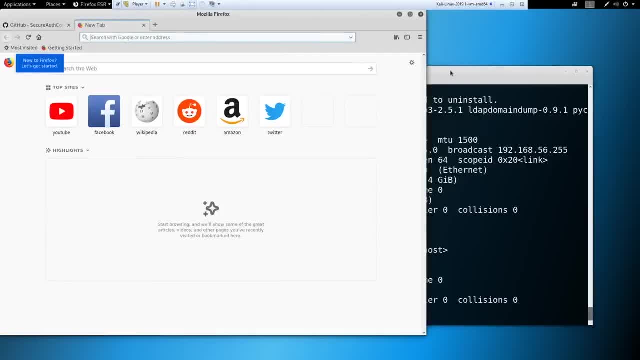 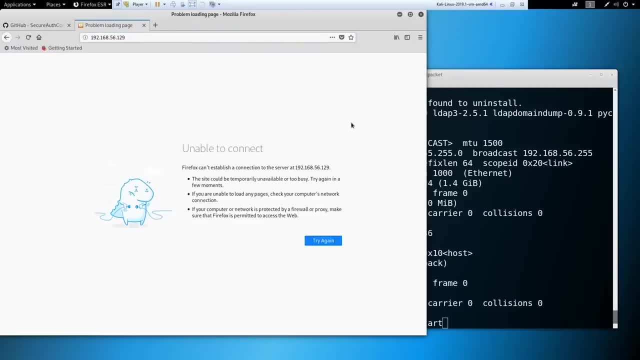 But before we hit enter, let's just make a proof of concept. We're going to go out to our address here, This 192.168.56.129,. whatever yours is, hit enter. You have a problem loading the page, unable to connect. 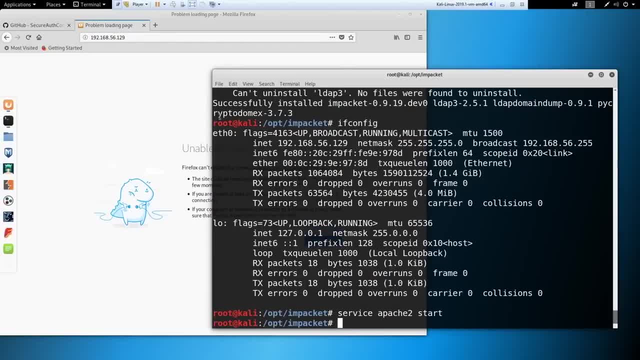 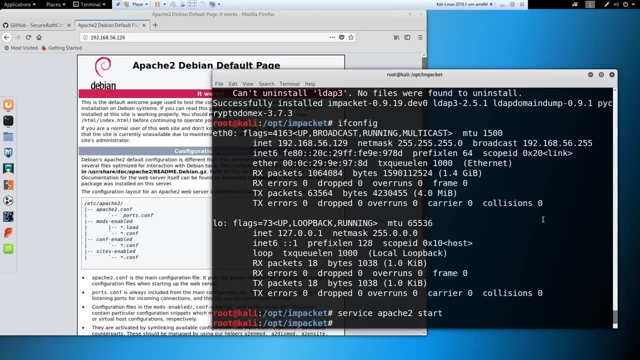 You're not running a web server. Okay, We'll say Apache, start, hit enter, and now we have a default Apache page. So it's as simple as that. Another one that would be good to start would be SSH, if it's not already running. 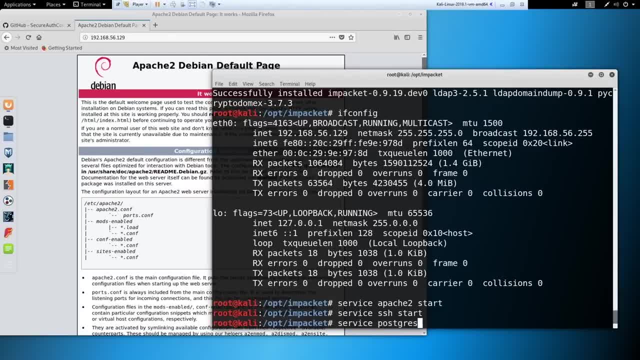 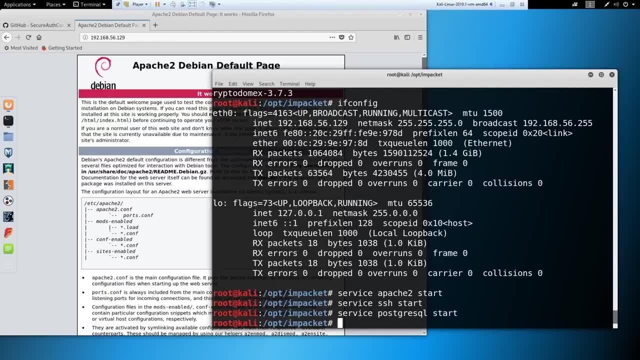 And service PostgresQL start, because PostgresQL runs with MetaSource. It's a very simple service, boy, and it's good to have that running Now. unfortunately, when you turn your computer off, all of these are going to go away. 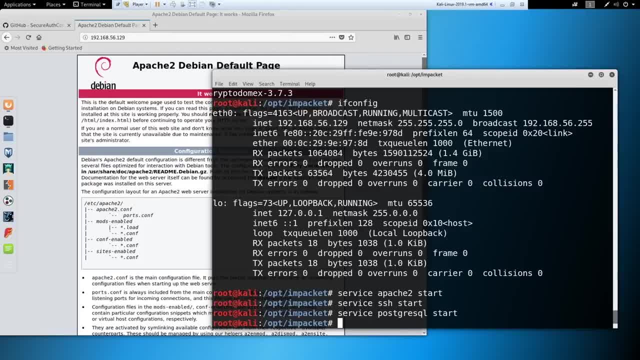 So what we actually need to do is we need to say systemctl, which Kev got ahead of us, and we're going to run an enable on this, So we don't have to set the Apache 2 to start, because I'm going to show you a better way to run a web server later. 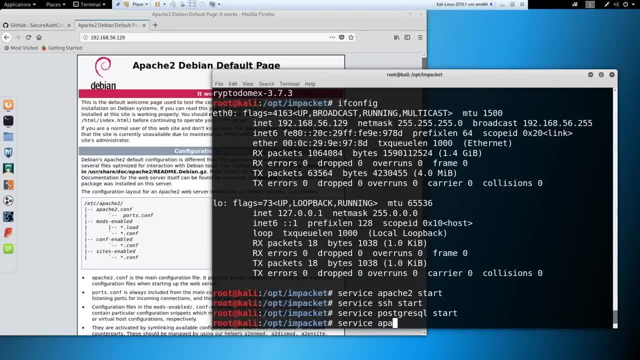 And actually I'll teach you while we're at it how to stop the service. So all we have to say is: service, Apache 2- start. So all we have to say is: service, Apache 2- start. So all we have to say is: service, Apache 2- start. 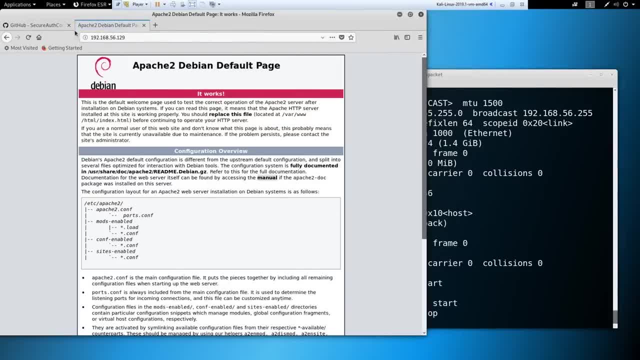 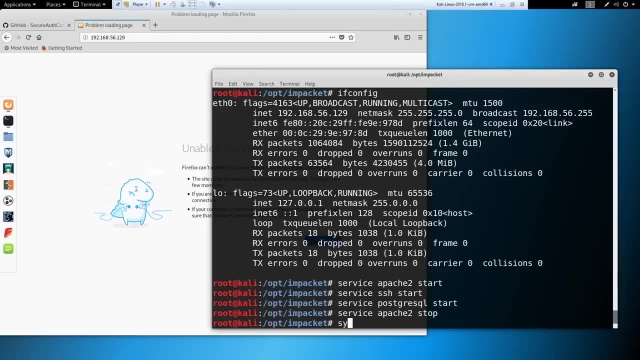 And then we come back in here and refresh and there's a problem loading the page again. So now we can use something systemctl, like this right Systemctl. we say enable and then we say, well, I won't say Apache 2, we'll say SSH. 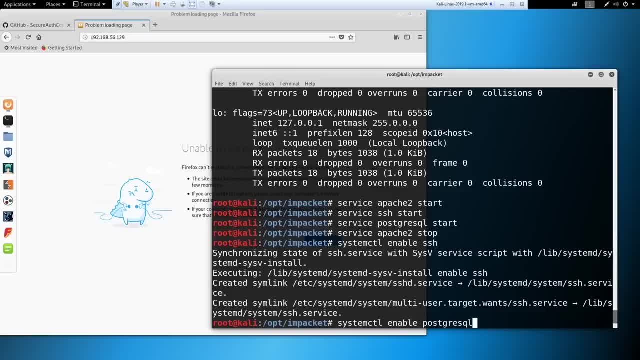 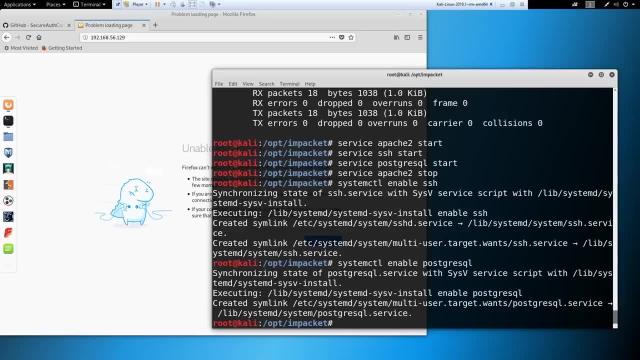 Okay, and then we'll say PostgresQL like that. Perfect. So now when we reboot our computer, these are guaranteed to start as well, So we don't have to start them on our own. So just a couple little things that may or may not be by default. 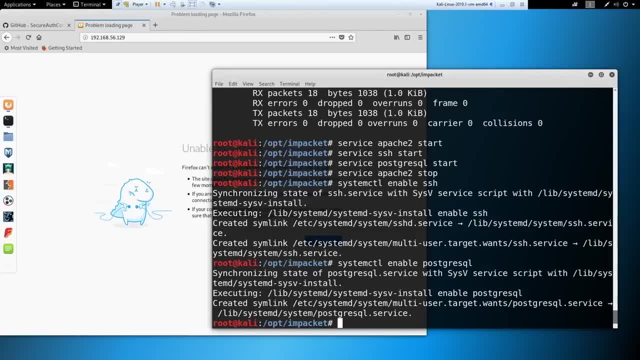 I have no idea anymore, clearly, what Kali is up to, So I'm behind on the times, guys. All right, I need to grab a drink and then we're going to get into what I hope is going to be the fun part of the course. 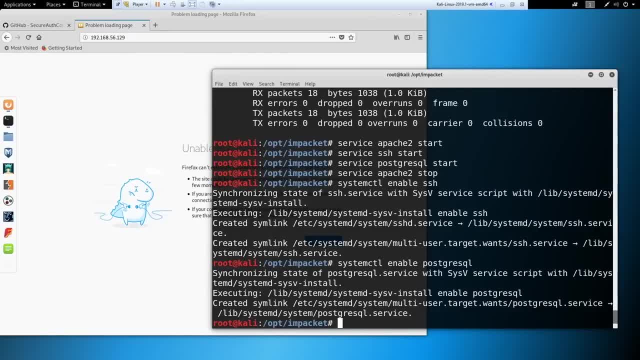 We're going to talk about scripting, We're going to write our own ping script here and we're going to do some cool stuff. Free drinks- You don't have to run SSH at boot. I run SSH at boot. You can do whatever you want in terms of being the security-aware individual that you are. 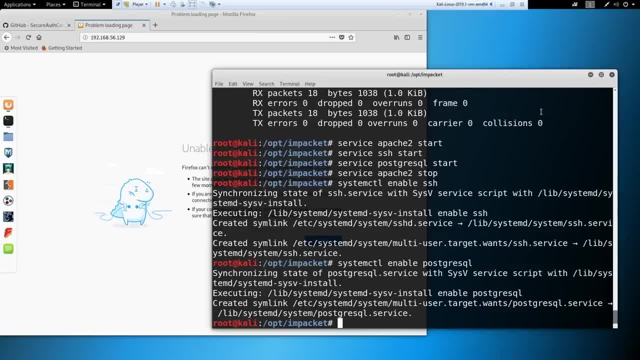 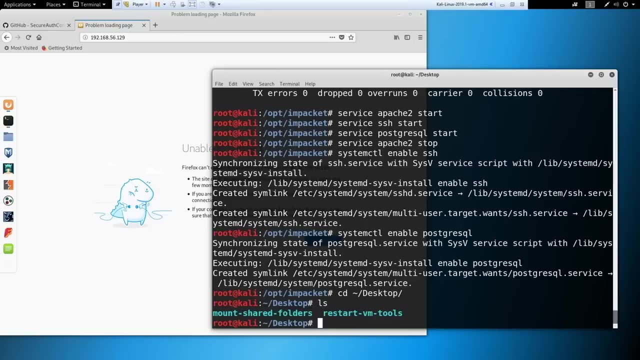 Sir or ma'am. Okay, So let's go into, Let's go to desktop. We'll do the Atilda desktop LS. Okay, So we're going to build out our own script. We're going to write our first script together, guys. 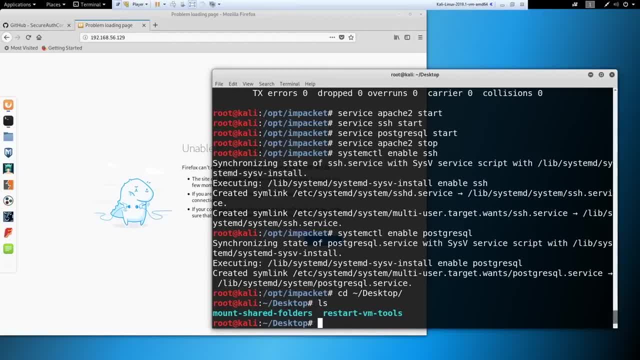 Monster Drink Frappuccino and DayQuil. That's hilarious. All right, So for our first script, remember when I said we were going to be dealing with ping. So we're going to say ping and then I'm going to ping an address in my house, like we just did. 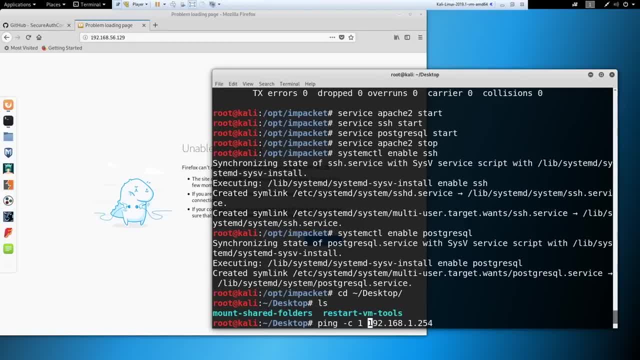 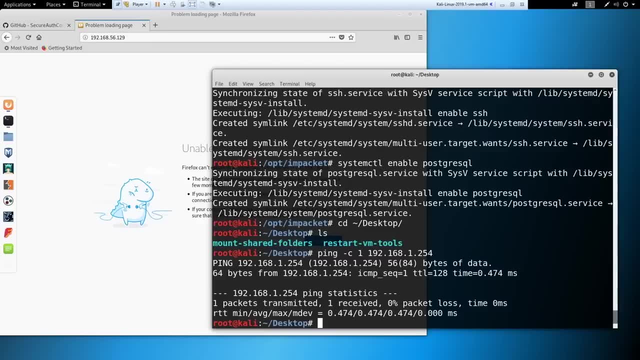 And I already showed you the count of one, so we'll just go ahead and do the count of one again. Make sure that address is up. Perfect, It's up. You want to see my pretty face? Why Nobody wants to see my face? 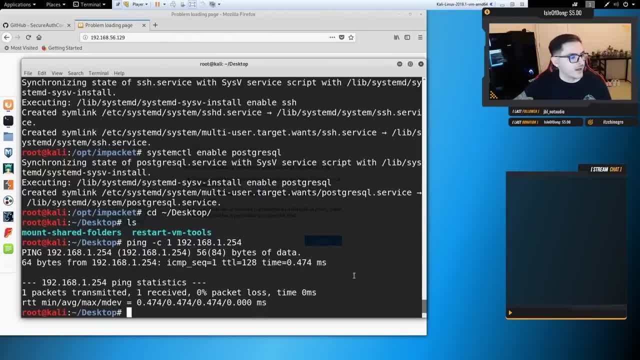 Boom, Hello, Hola. All right, So here you go. So when you come in here, let's go ahead and tab up on this, and we're going to write this to a file. We'll just call this iptxt. 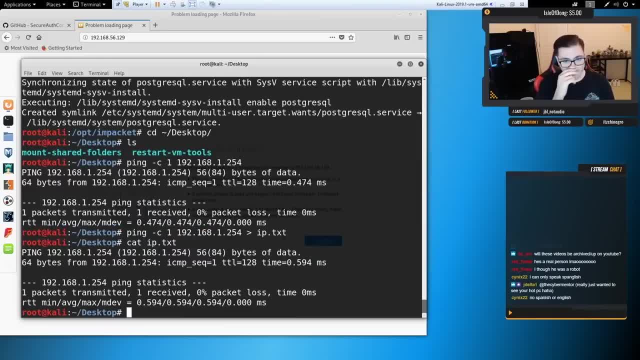 So if we cat iptxt, we'll see here that we've got the same information from the ping that we just had. Okay, So what we're going to do is we're going to break this down and we need to extract this information. 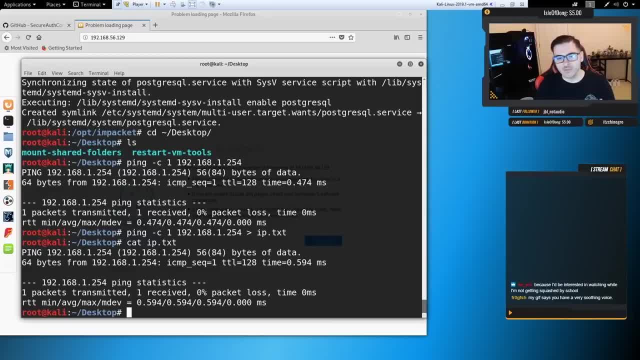 So our goal here is that we're going to build a ping sweeper. By that I mean, we're going to build a script that goes through this IP range of 1 through 254, and it sees who's up, right. So right now we know for sure that this guy is up. 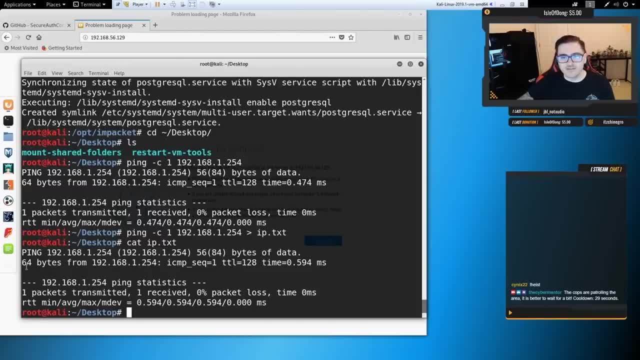 Well, how do we know that this is up? Okay, well, it says it received 64 bytes from 192.168.1.254.. Okay, well, what if I ping count of 1, something that I know is not up? 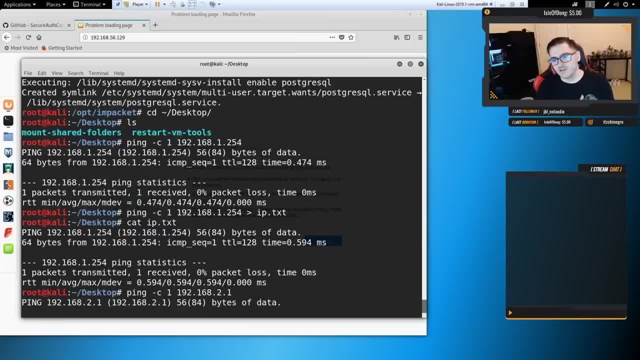 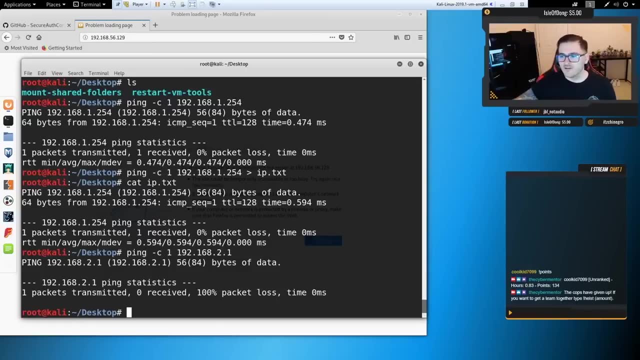 We'll do 2.1.. We'll try to ping that. Well, thanks, Nate, I appreciate that. Tell your girlfriend I said thank you. Tell her I said to adopt my kittens, All right. So you see when this ping comes back unresponsive. 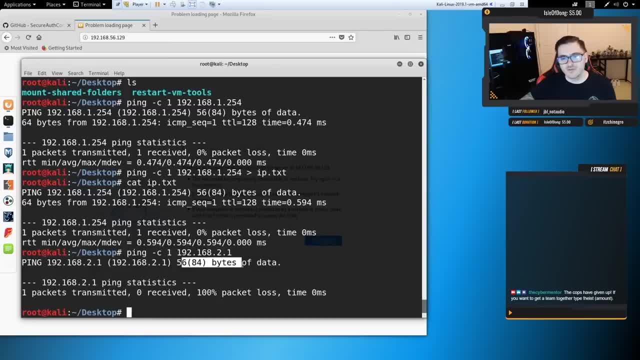 there's just no bytes of data, right, It's got the 84,, 56,, whatever this is, but it doesn't have this line here. So this line is the difference. So we want to differentiate between a up machine and a down machine. 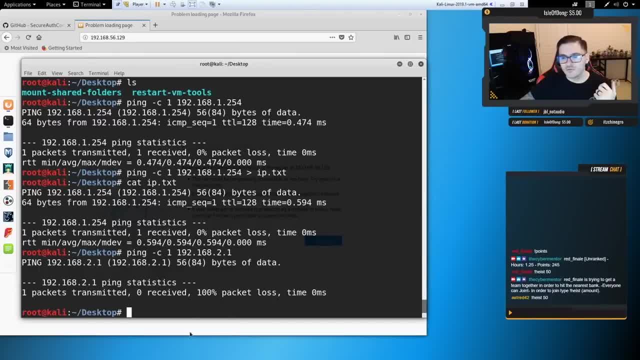 We do it by this line. So when we come into here and we have our cat IPtxt, the first thing we're going to want to do is we're going to say, okay, what's unique about this line? Well, if we look at it, this IP address is everywhere. 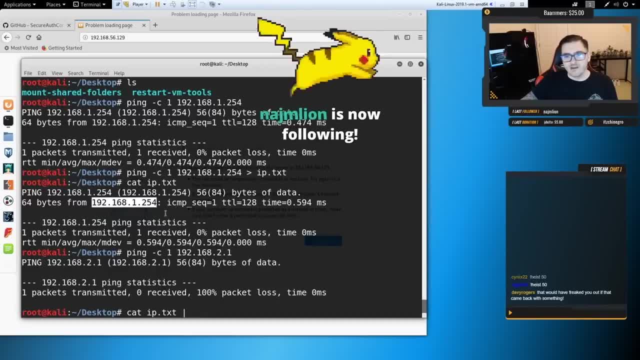 So it's not really the IP address that's unique through this line, right? Maybe the sequence here, this ICMP, might be unique. Okay, There's some other things that are unique that we can kind of grep off of. What we're going to do is we're going to grep. 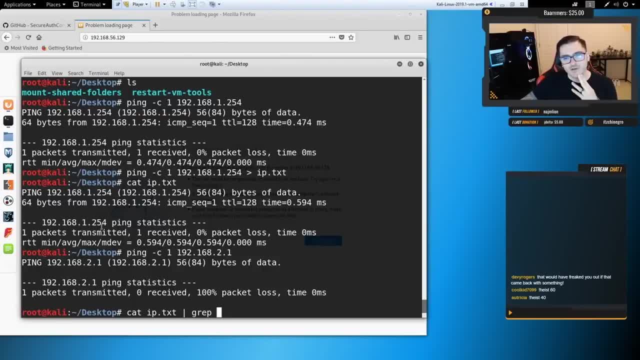 and we're just going to build off of this script. One of the things in here that is greppable is this: 64 bytes right here. So we're going to say: yeah, Davey, that would have freaked me out if I came back with something. 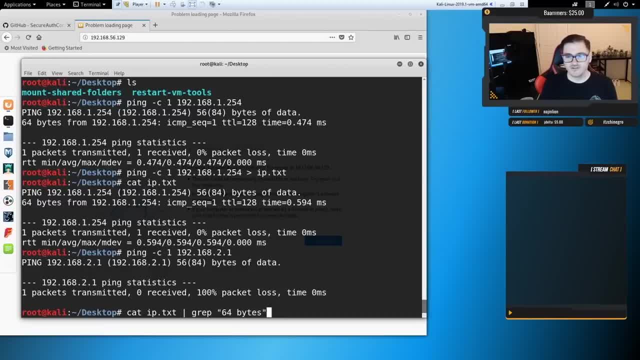 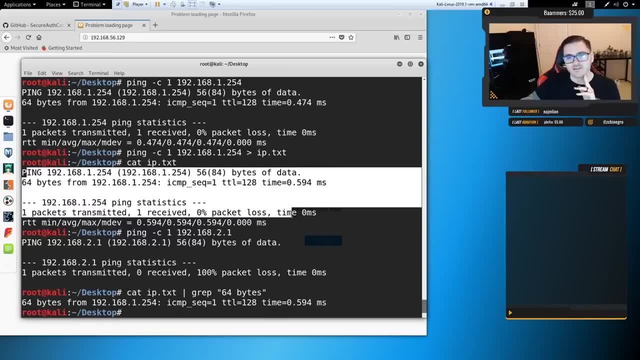 because I should not be attached to any network. So if we grep on the 64 bytes, you can see now that from this whole IPtxt I just pulled out the 64 bytes. So this one line right here. Okay, I really want to narrow this down. 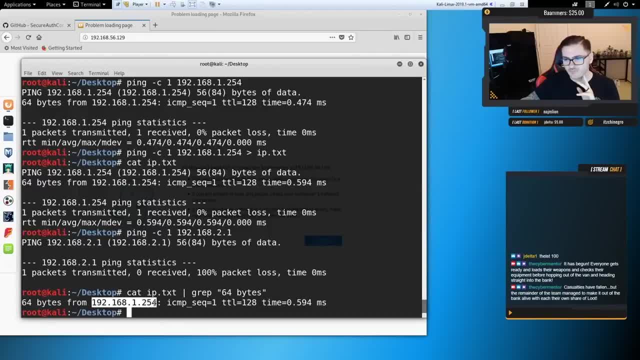 All I want to get out of this is this IP address here. I'm trying to get this IP address so we know what IPs are talking back and what IPs aren't. This is the whole point of the ping sweep. So we've grepped. 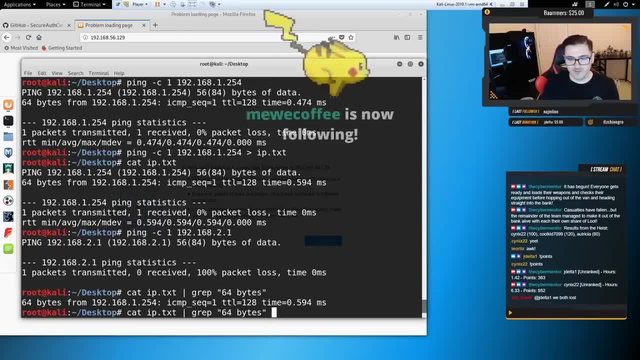 We've added a pipe and a grep and a grep just pulls out the line. We're going to add another pipe and do another command here. What we're going to do is we're going to do a cut, Now a cut, and I'm going to type this out real quick. 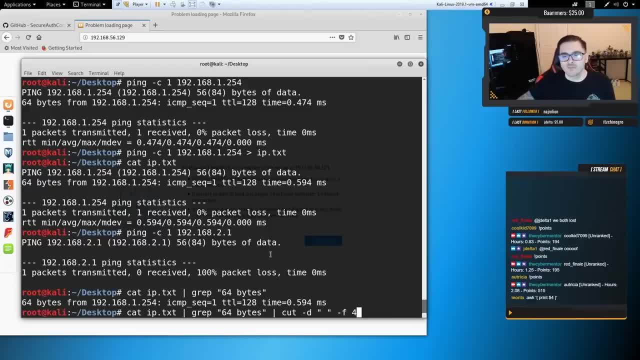 is going to take a delimiter and the delimiter here is a space, and then it's going to pick a field of that space and cut that out. So this delimiter, okay, a space, and it's a field of four. So we've got a space here: one, two, three, four, right? 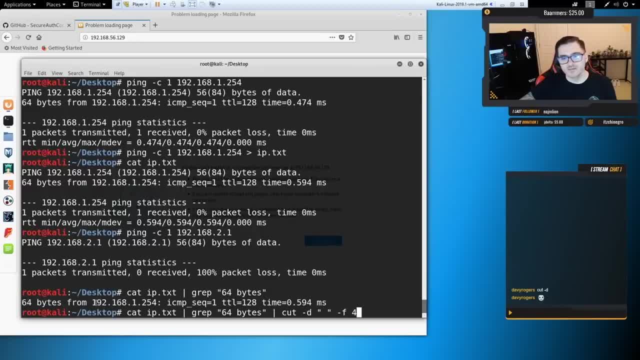 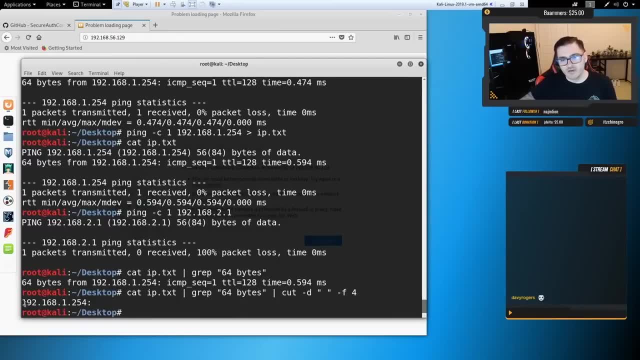 So this is our fourth field. One space, two space three, space four is this field. So when we cut this and hit enter, we actually cut out everything except this. Okay, So when we have an IP address, the last thing that we have here is we've got this. 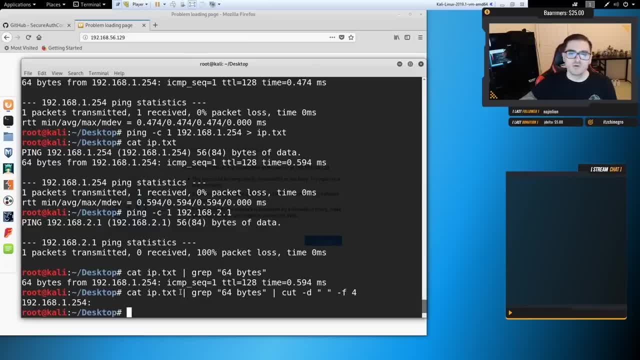 little colon that we do not want attached to this IP address. Well, we can do a few things to remove it. We could use sed. I actually like to use tr, So tr stands for translate, and all we have to do is say translate. 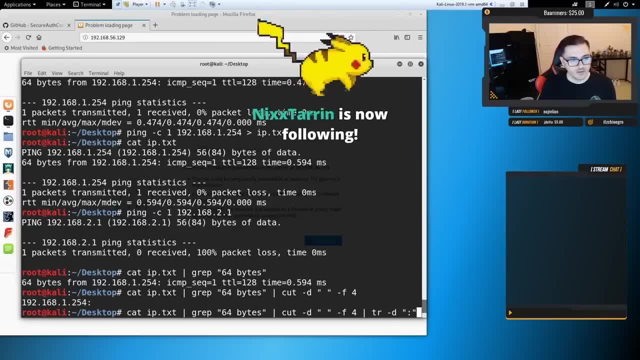 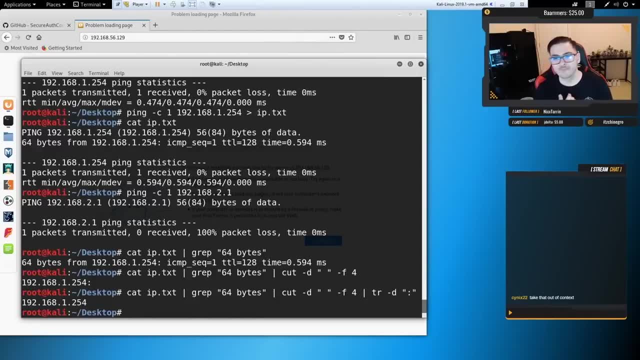 with another delimiter, We'll put the colon in and then we'll hit enter and it removes it. Okay, So now we have our IP address. So we've kind of built out the product that we need to send this into to a script and make it work. 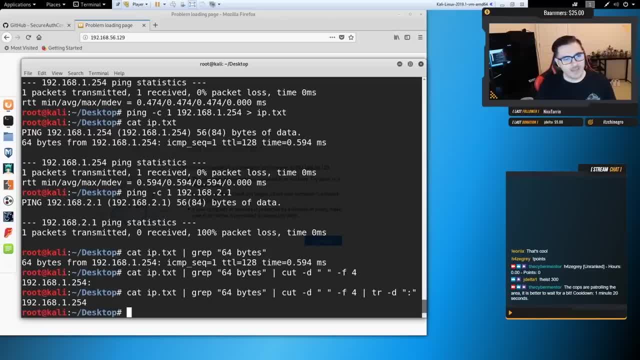 Okay, So now we're going to build our first script. I was going to build it in gedit because I like to build in gedit, but apparently that's not going to work. Hey, thanks, Conrad. I appreciate the sub. 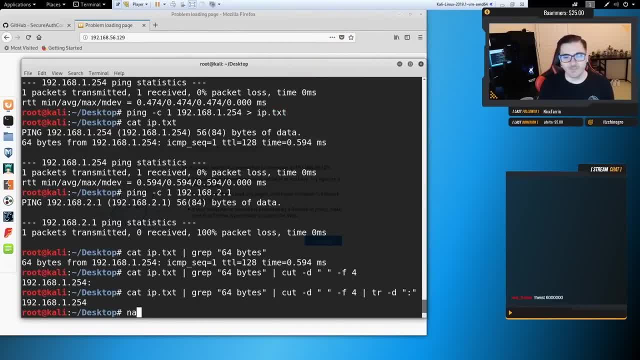 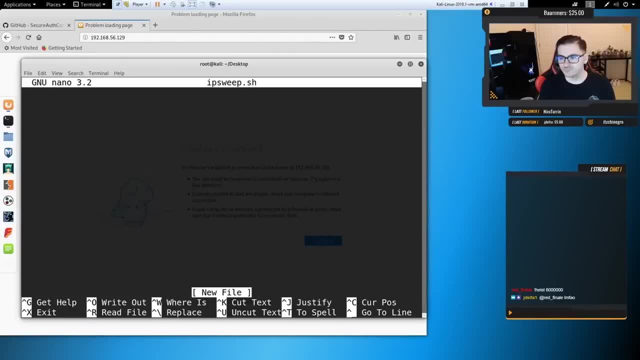 Since it's not going to work, we're just going to use good old nano and we're going to call this ipsweepsh. Okay, Now, at the very top of any script, we need to declare what we're running. So if this were Python, we'd be running bin Python. 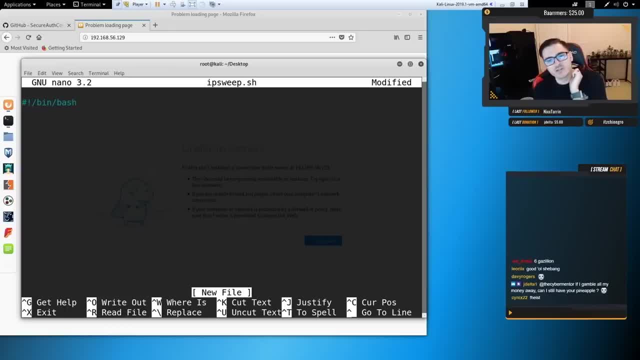 but here we'll actually be running bin bash, And we'll cover this more in depth next week when we start talking about Python. But for now, just know that at the top we're going to be declaring the bin bash location and that we're running this in bash. 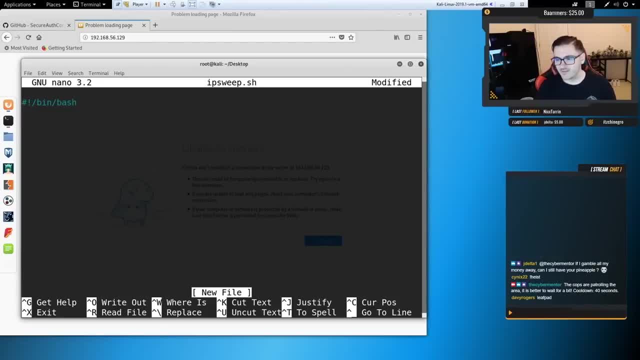 This is going to be a shell script, hence the sh, You guys, and LeafPad. Okay, Bye-bye, Bye-bye, Bye-bye, Bye-bye, Okay. So we're going to do something called a for loop. 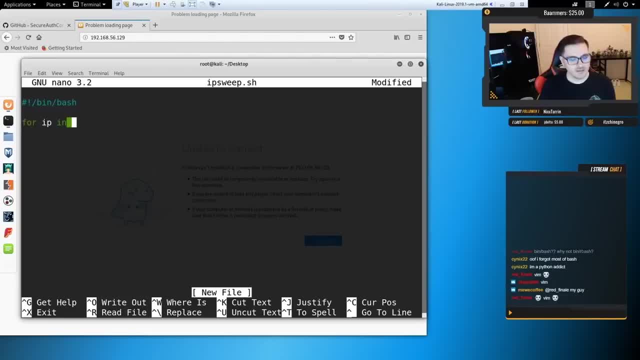 And let me type it out here. So we're going to say for ip in sequence, And note what's in front of sequence: It's the little thing next to – I don't know what that's called: The thing next to one. 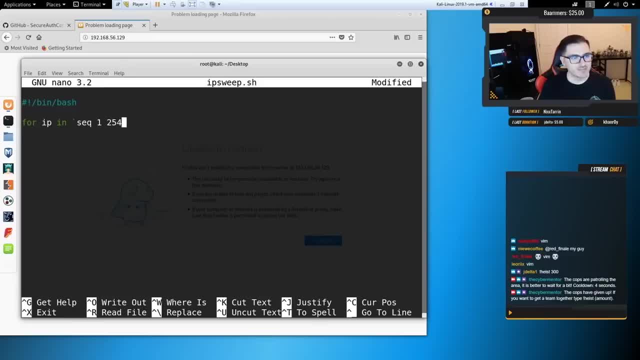 If somebody knows the name of that, please educate me. You guys have been doing it all night: Back tick. It's not the Attilda. the Attilda is the, the shift version of that back tick. you guys are awesome. All right, Let me type this out real quick and then I'll explain everything that we're doing. so if you want to follow along as I type, 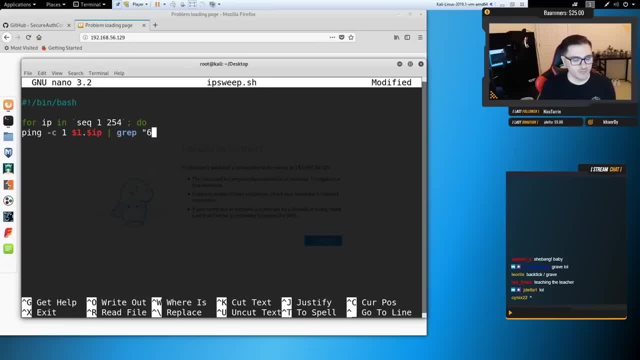 this out, But most of this should look really familiar. So I'm going to do a for loop and I'm going to do a for loop, and I'm going to do a for loop and I'm going to do a for loop. Okay, Teaching is absolutely the best way to learn. 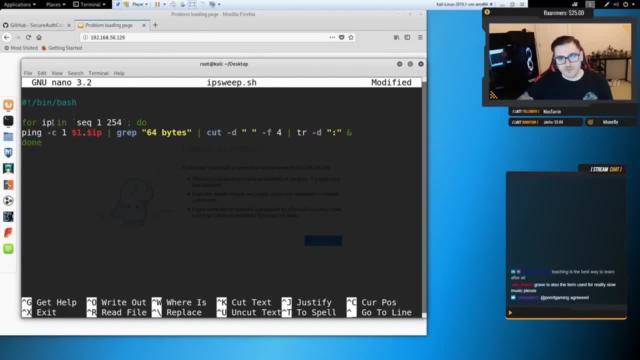 Okay, So we're doing a for loop. So we're we're doing a for loop, We're saying for something in something here, We want to do something until it's done right. So for an IP address, and this is just a variable that we're declaring. we're declaring. 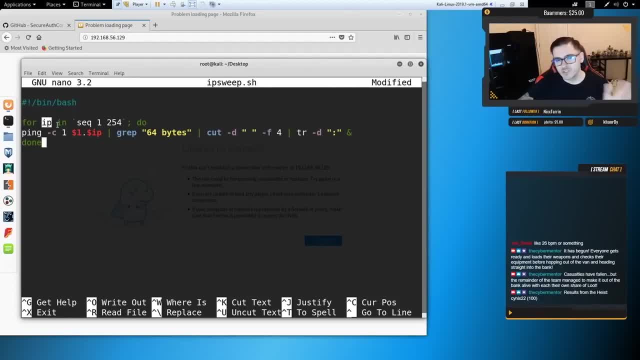 IP. we could call this whatever we want, but we're just calling it IP for now, for IP in Sequence 1 through 254.. So that means we're gonna run through one all the way through 254 and We're gonna say, okay, Well, when we go through that sequence, every single time we go through this sequence in this loop. 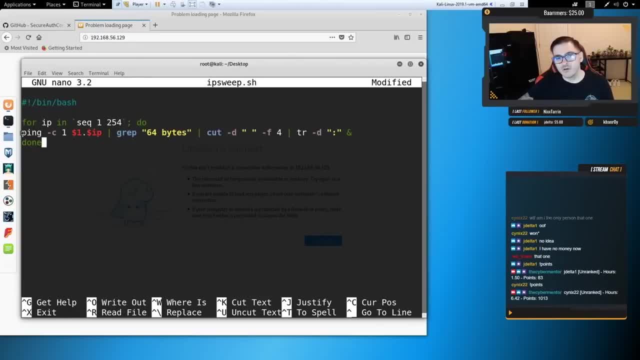 We're gonna do something. What are we gonna do? We're going to ping a count of one dollar sign 1, Dollar sign IP. Okay, What does this mean? dollar sign 1 is user input, And what that means is, when we run this script, we call this IP sweep. We're gonna run it like this: IP sweep sh. 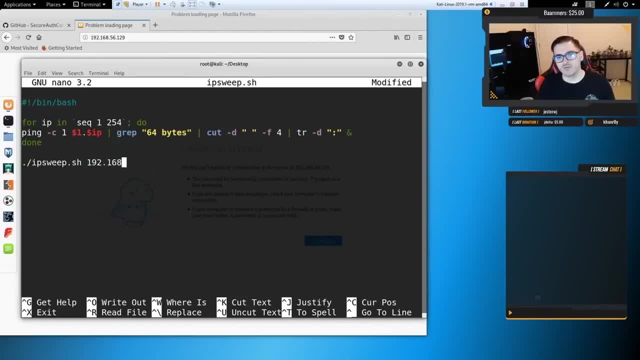 We need to call something. so I'm gonna call out something like this, because this is the first three octets of my network, right? So I'll call out 192 dot, 168, dot 1, and then we'll have a dot here and then the IP. 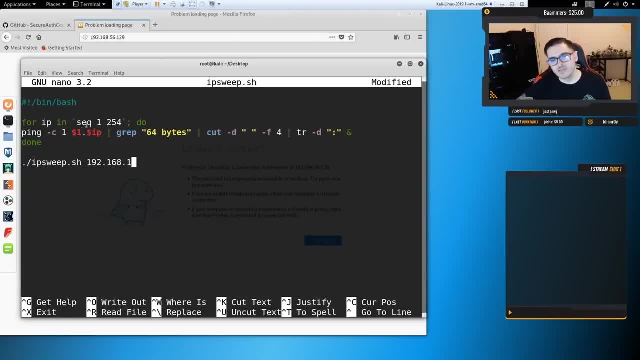 Remember we declared IP right here, So the IP is the sequence 1 through 2? 254. so every time that we sequence through this loop, We're going to be saying 1, 2, 3 on this: 192 dot 168, dot 1. 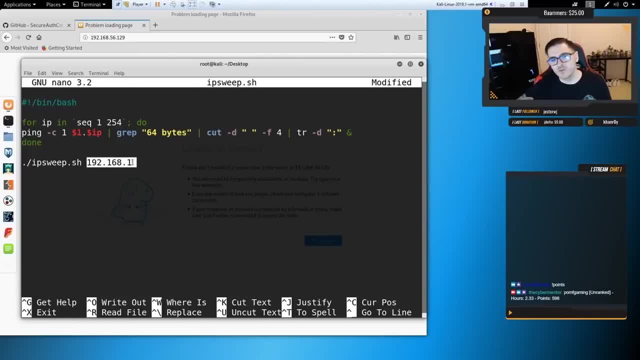 We could also remove dollar sign 1 and hard code this if we wanted to, and then it would just run through this. This just allows a little bit more flexibility, allows us to type it in, and if we're doing a different network or whatever On the fly, we could just use this quick little ping sweep. 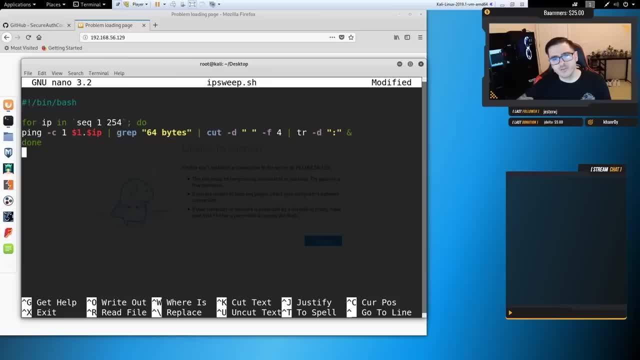 So, anyway, I'm going to delete this out Now. the rest should look fair, Fairly familiar. Okay, you're going to grab 64 bytes, cut with the delimiter of space to a field of four, and you're gonna translate. now The only thing: yes, control K to delete line. I did know that, actually that I did know. 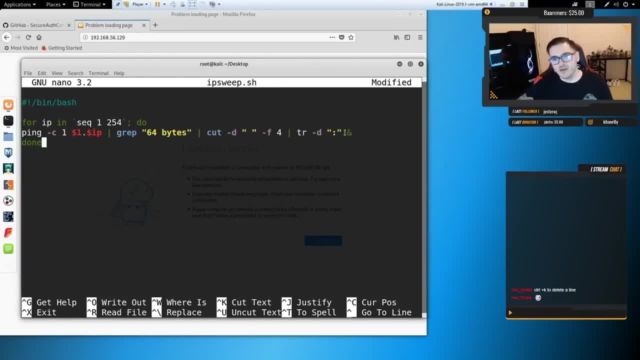 So here there's two options that we have. You could put another semicolon after the parentheses here and say done. What I like to do is add this ampersand. the ampersand allows us to do threading, so Instead of pinging one at a time- 1 through 2, 54- and figure out what's up or what's not up. 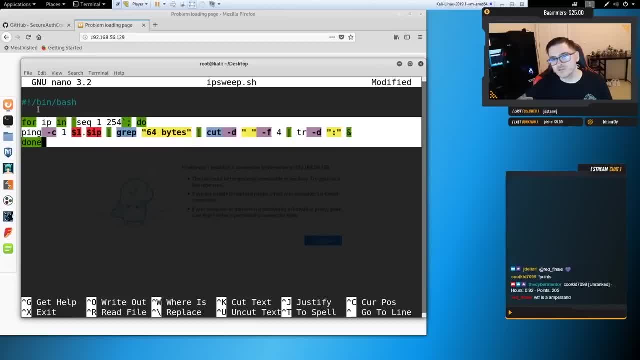 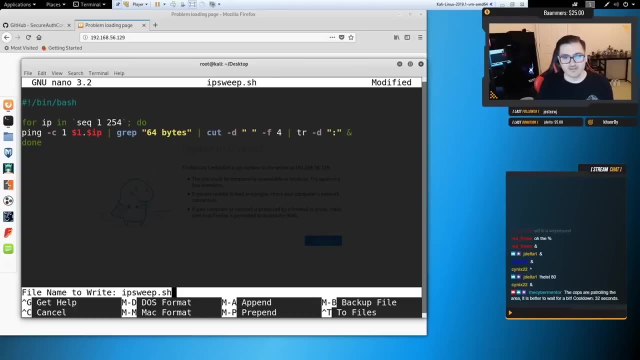 What we're gonna do instead is we're gonna ping them all at once with threading, So it allows us to finish it really really, really quick. So this is the very, very basic version of this. So let's go ahead and just hit ctrl X, Say yes, enter. 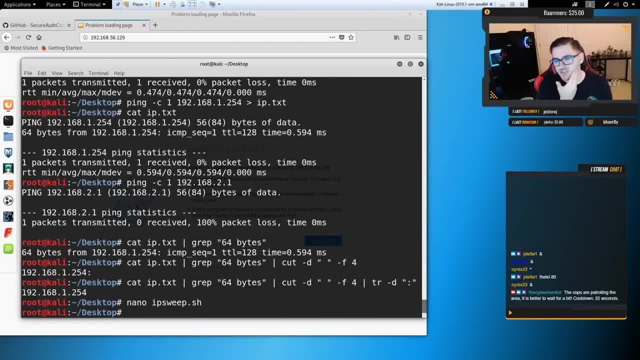 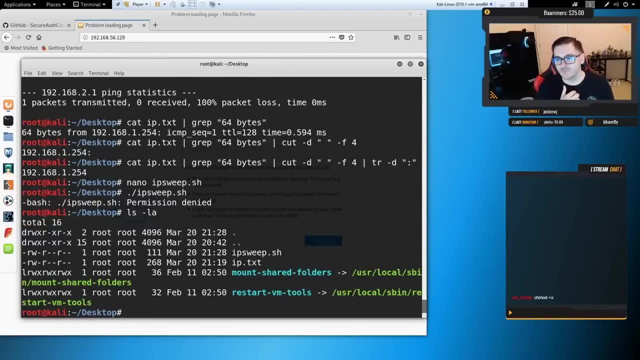 now, if you guys remember from earlier, I said that change mode would come back to be important. Why? Because if I say IP sweep and I hit tab, tab, tab, tab tab, I cannot autocomplete Permission denied. We do not have execute permission on IP sweep, So we need to chmod plus x And then we'll say 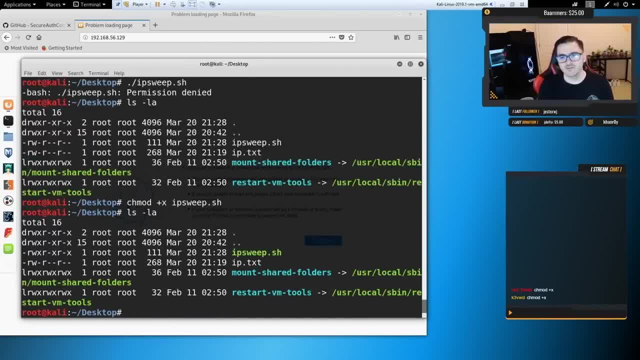 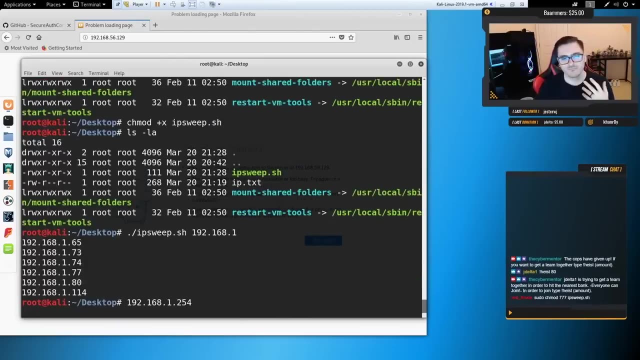 IP sweep: LSLA again confirm, Perfect, Okay. so now what we need to do is we need to enter in our first three octets And then hit enter Okay, so it returns those IP addresses. and it's still threading right now, So it's still going. 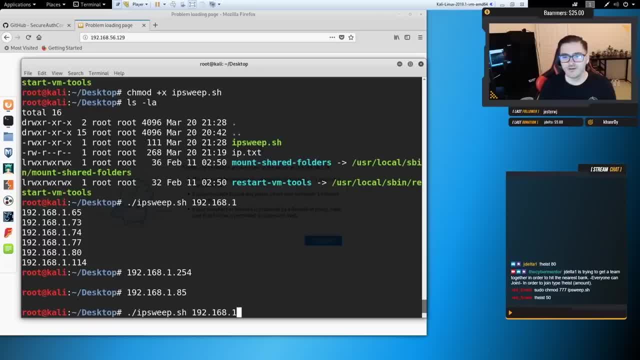 through, And if we want to do that, we're going to hit enter, And then we're going to hit enter, And if we want to even do one better, we could say: IP listtxt, Run it through, And then you can. 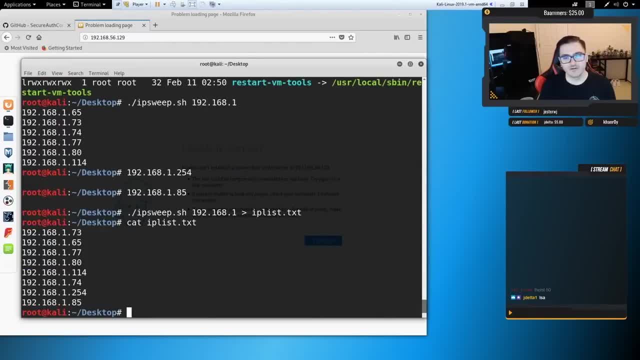 cat the IP listtxt And you have your list of IP addresses that are up in your network. So it goes by pretty quick. Now we can improve this a tad bit. If we forget, say, for example, our IP address- 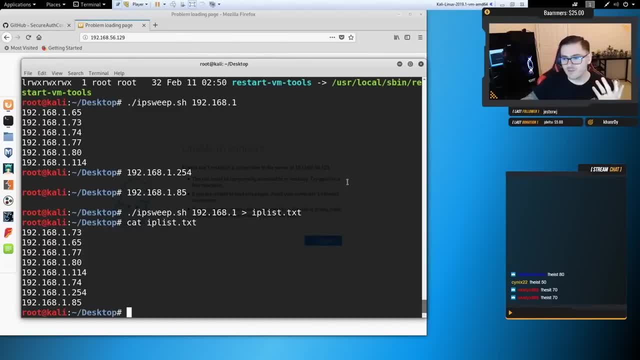 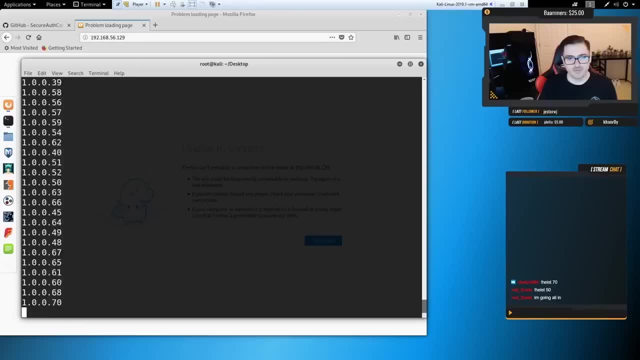 or say we forget to type something in here and it gets a little funky, Like if we. I don't know what this is going to do to me If I mess up or I just type in one, okay, it's going to type 1000255.. Right, And it has no idea what's going on. 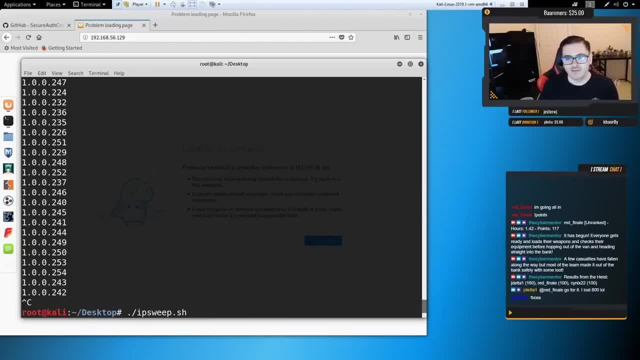 So say we do, that we forget to type something in. This isn't going to be perfect by any means. All this is going to allow us to do is just add in some little bit of filtering. Okay, If you get better at coding and scripting or whatever, you'll learn how to edit these down. 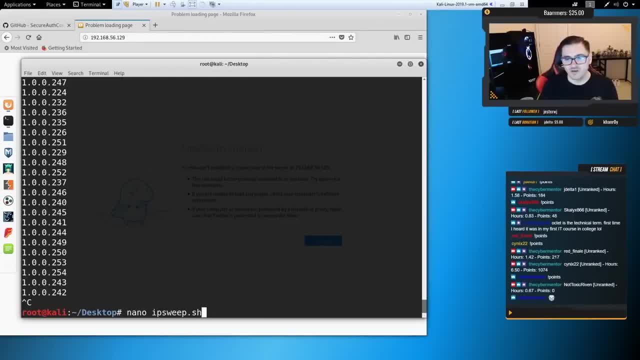 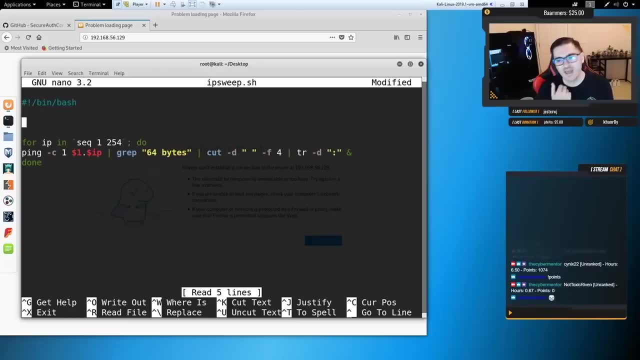 and make these more protective against these measures. But let's go back into nano- And I take no credit for this. I learned this. I've modified this just a tad. I think this came from Georgia Weidman a long time ago. So very, very straightforward, very good lesson to teach. 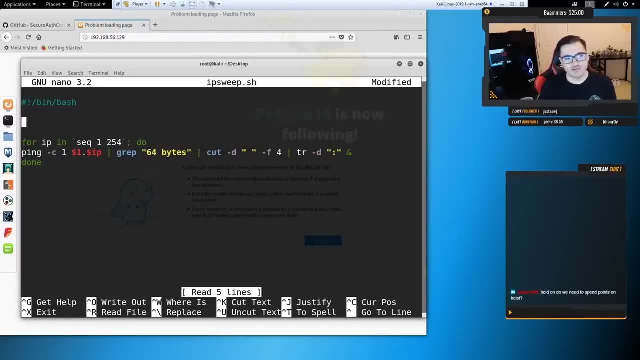 out. So what we're going to do is we're going to add an if else statement And we say if, and we're going to add a condition. The condition is, if dollar sign one is equal to blank, then what are we going to do? Well, we can say: echo you, for I can't type guys. 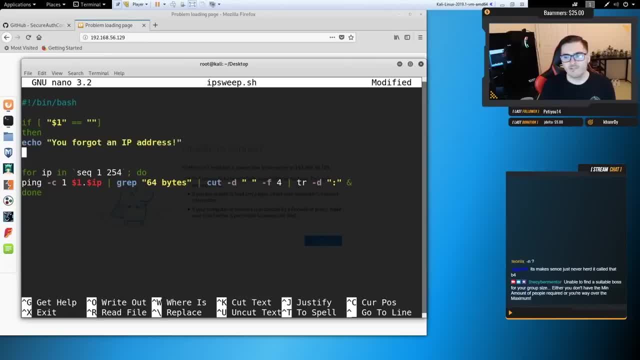 you forgot an IP address. We can also echo the syntax out. We can say: syntax: IP sweep, shsh. And then you can give an example right here, right, Okay, but say we did provide something in dollar sign one. then we say else, go ahead and ping this. And then we'll say: fi. 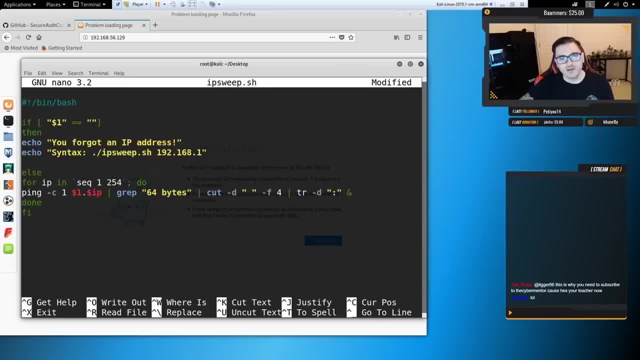 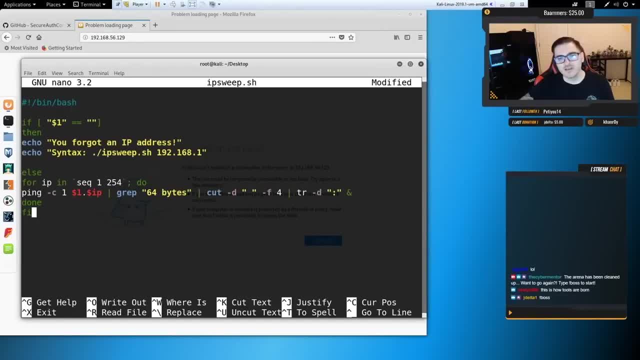 this 192.168.1 is not present. if there's nothing present there, then you're going to say, hey, you forgot something. Else you're going to go ahead and say, okay, let's go run through this. 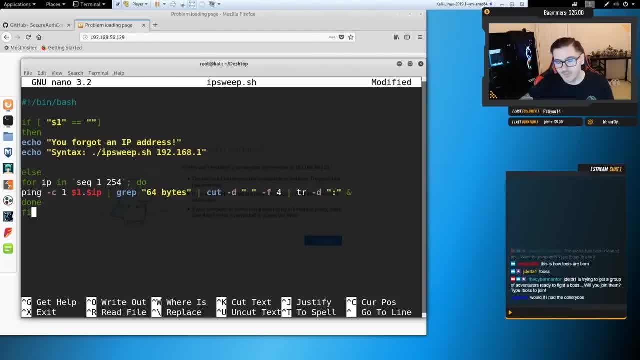 And then we're going to end the if statement with if backwards, which is fi. Now, obviously we could get better at this, Because if we don't put in three octets or whatever, this program is not perfect. This is just a very basic ping sweeper, Not something that you would. 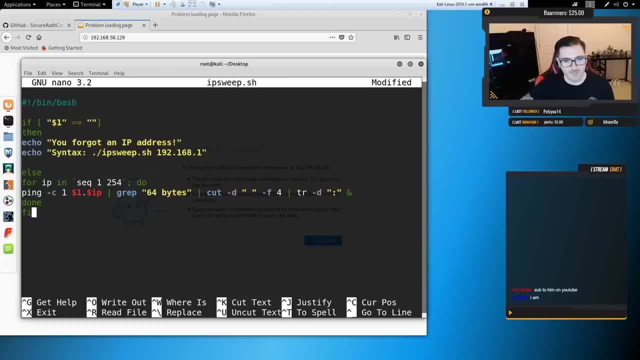 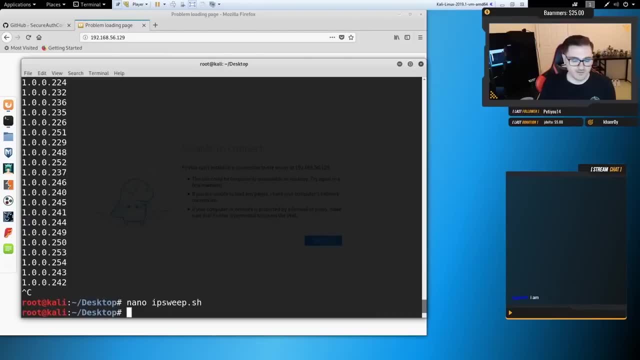 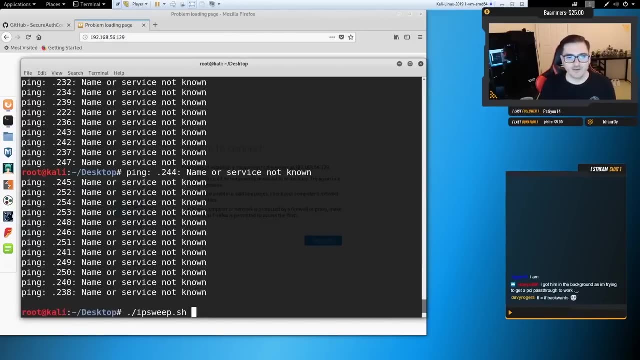 release to the public or anything like that, because it would break very easily. Anyway, we hit Ctrl X on this, We hit yes to save. Now if we try to run IP sweep and we forget to put input, apparently it still runs. I don't know why that does. 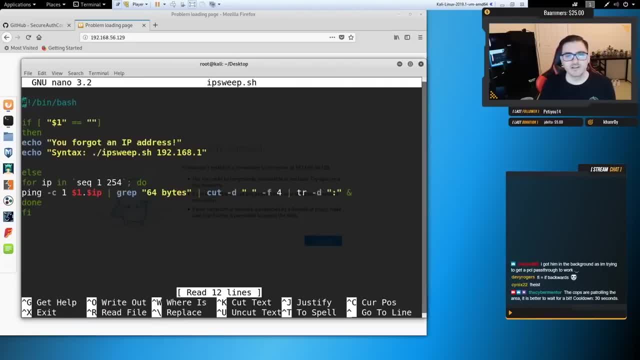 What did I break, guys? What did I break? It's a learning lesson together. Does this need a space? If then else end, I think we're good. I broke the script, Guys. I broke it. There you go. It needed a space. Syntax is everything, ladies and gentlemen. 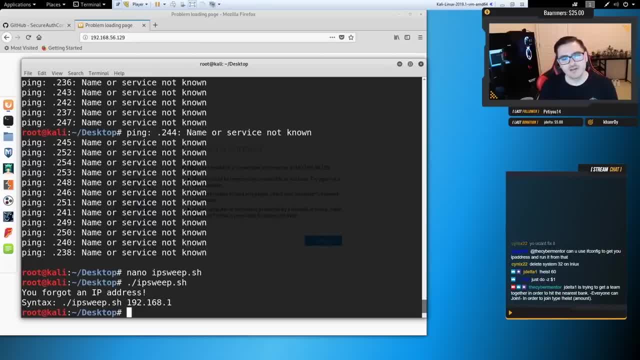 So here you go. You see, now it says you forgot an IP address And it gives you the syntax. So it's just a little added measure to do this. So now we're gonna go ahead and take what we've learned and we're gonna throw it into one last. 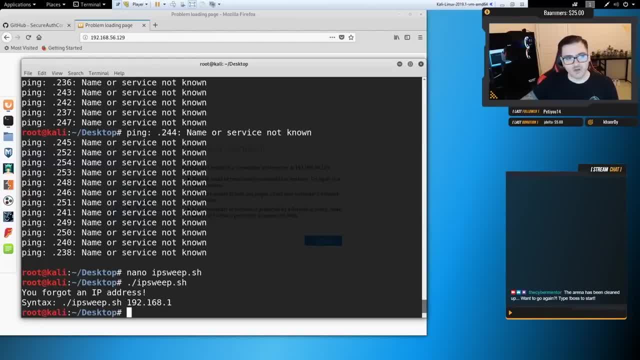 thing And these are really useful. So these are what we call one-liners, and that's where you write everything out in one line from your terminal. So, for example, we have this IP list right, This cat IP list. 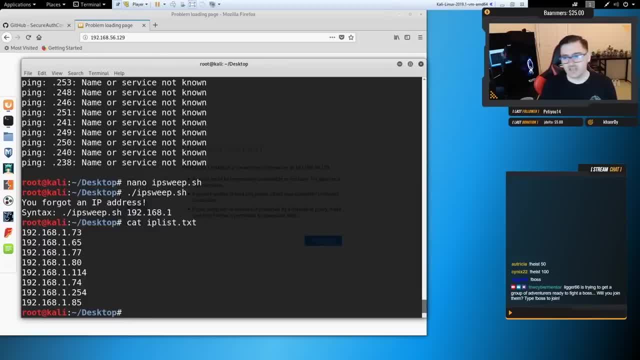 Let's see what that is. Say I wanted to do something with this IP list. Okay, say I wanted to run an nmap scan And with that nmap scan I want to scan every single IP in this IP list. Okay, well, a quick way I can do that is I can say for IP in: 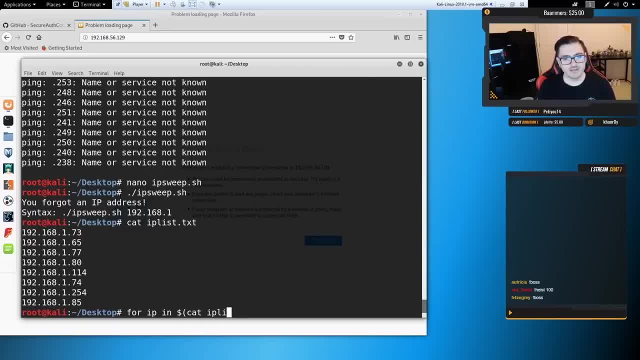 and then we'll say, $cat, IP listtxt. And then we can say: do nmap. And you guys don't need to worry about this right now. We'll say: let's just scan for port 80 on all of these machines, $ip and done. 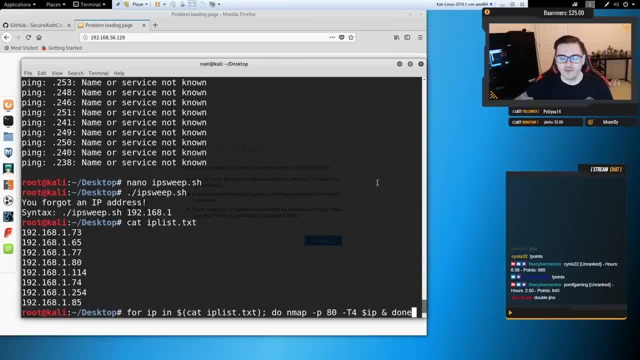 Okay, so it looks very familiar, right? What we're doing is very similar to what we just did in the IP sweep, but we're doing it in one line, So we're saying okay for IP. remember again, this is just a variable. 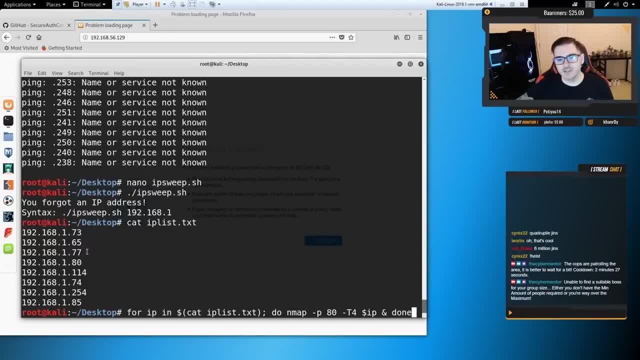 In and then we're going to cat out this IP listtxt, So it's going to go through every single one of these that we have in here. Okay, we're going to do something for every single one of those. We're going to say we're going to run nmap. 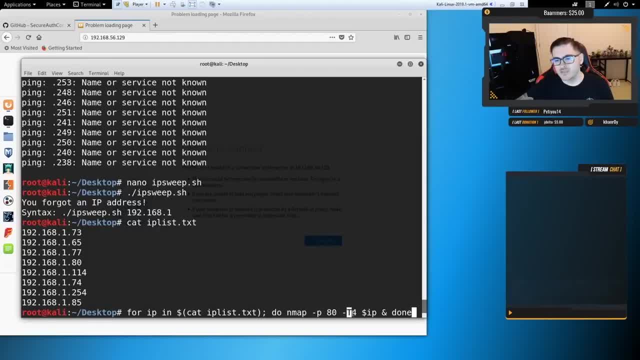 We're going to only be scanning for port 80. We're going to run at a speed of T4, which we're going to cover this later- in scanning. If you don't know anything about nmap, don't worry. Here's where we pull in the IP address. 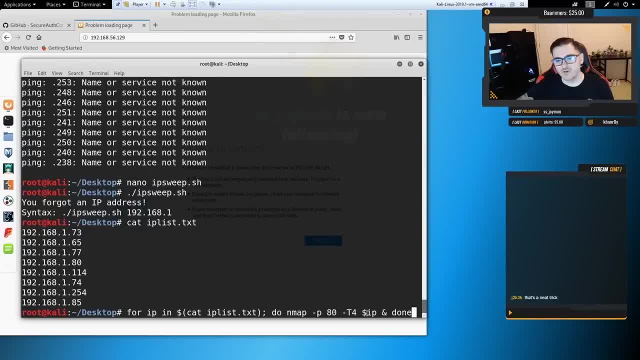 So we declared IP here. Every single one of these are going to be thrown into right here, And then we're going to say and done Okay. and then if we hit enter, remember the ampersand here runs them all at once. 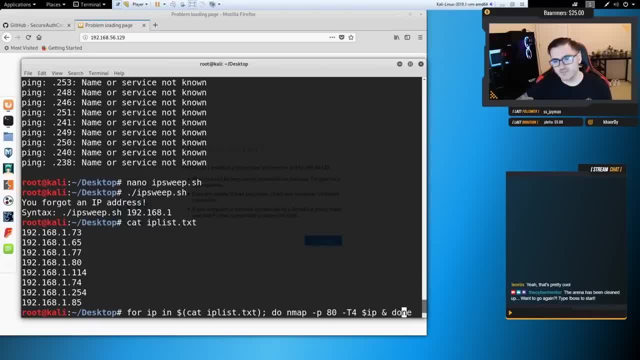 If you prefer to run them one at a time, you can delete the ampersand and just say: semicolon done. I like to use threading if we can. It makes it a lot faster. Okay, and now it's going to run through and it's going to say what's open, what's not open. 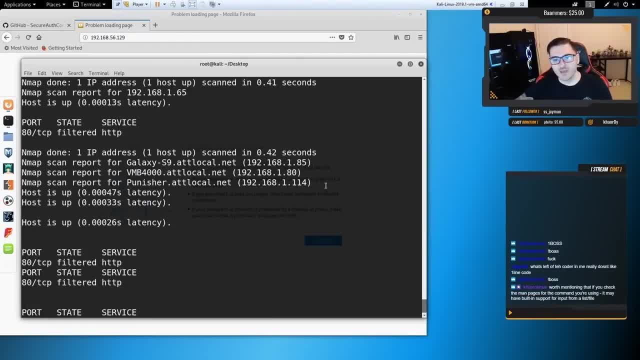 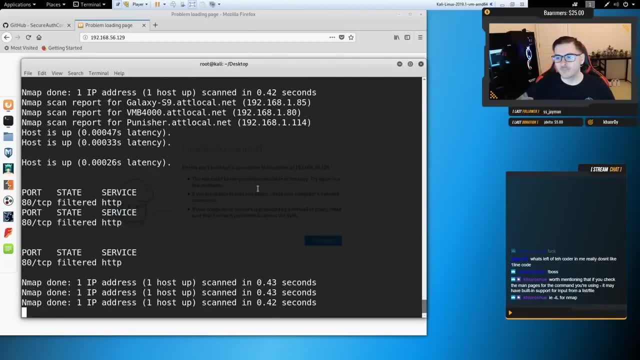 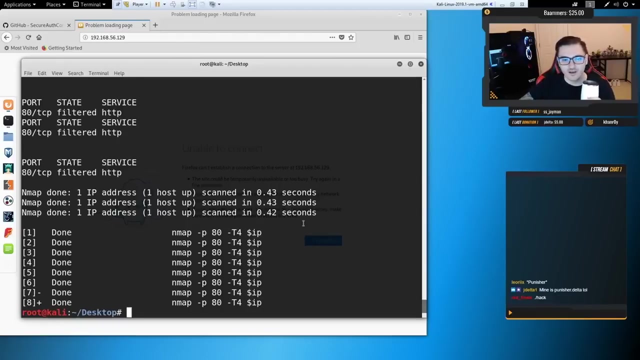 Oh man, you guys are getting my host names. Shame, You're really going to hack me now. Yes, the man pages are always worth mentioning. If you don't know that, I love the Punisher, you know now? Yeah, so you can come through here and you can kind of like look through these reports. 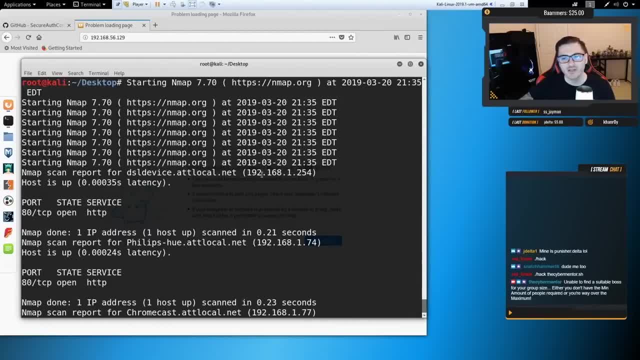 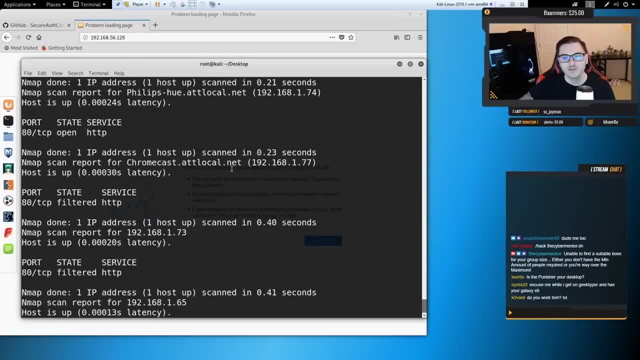 It kind of starts them all at once, which is weird, but then as they finish it lets you know like: okay, 1.254 has 80 open. 74 has 80 open. The Philips Hue has 80 open. 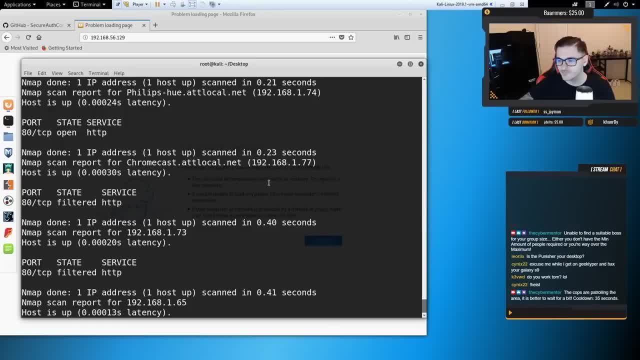 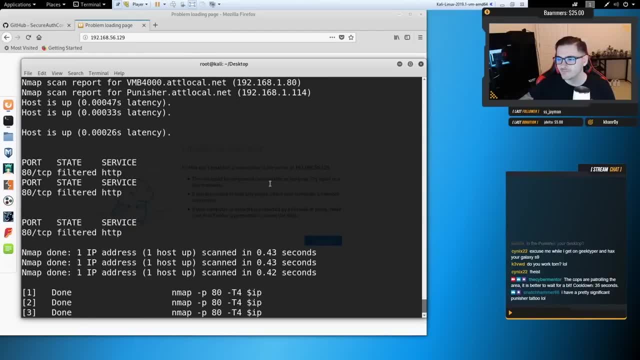 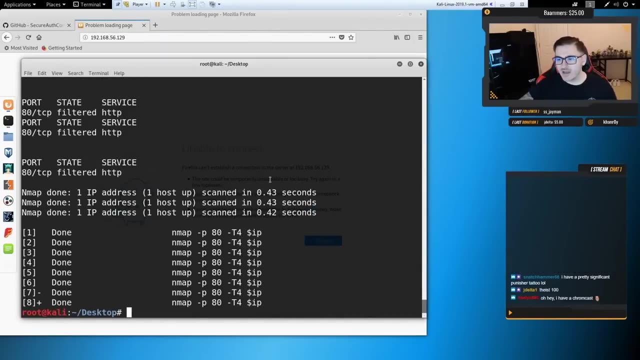 That's nice. The Chromecast has 80. open Is Punisher my desktop. Punisher is my desktop. Punisher is my desktop. I have a pretty significant Punisher tattoo my friends. Hey, you want to see my chest. 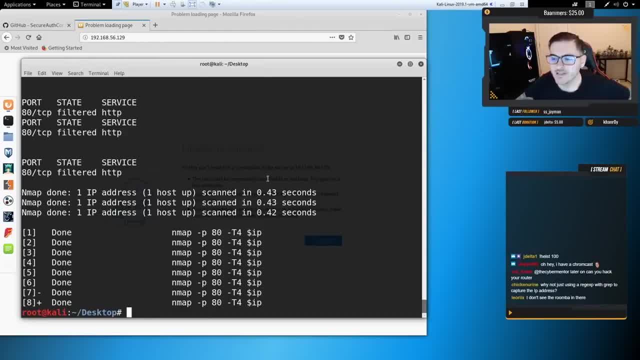 Look at that, guys, And you didn't think I was going to get naked tonight. Snatchhammer, I think we're friends, buddy, I think we're friends. Are there any exploits that would be used to the fact that these are? 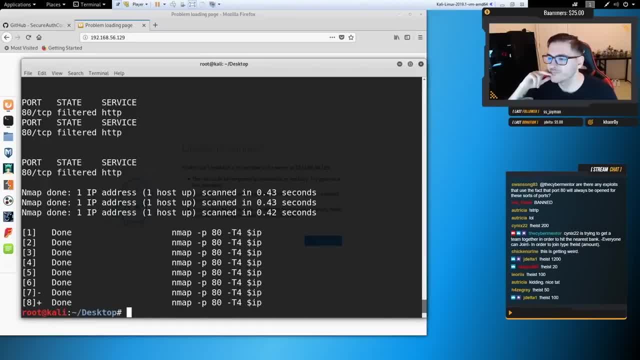 Maybe you would have to do more scanning and enumeration to know So, But that's it, guys. If you guys want to ask questions about this or anything in particular, I'm going to open it up. We actually finished 20 minutes early for AMA. 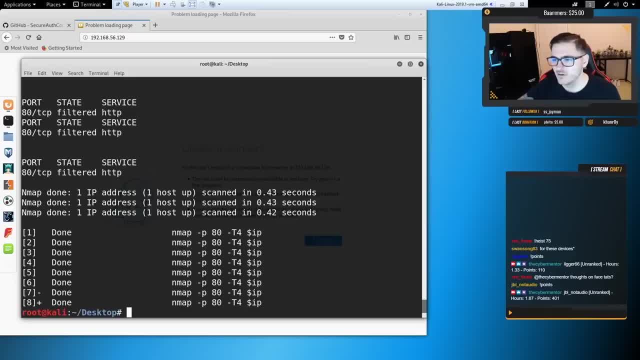 So that's all I've got for you in terms of Linux for this week. And remember, this is just. This is just introductory Linux. This isn't all the Linux that you should know or will know. You're going to come across more as you go. 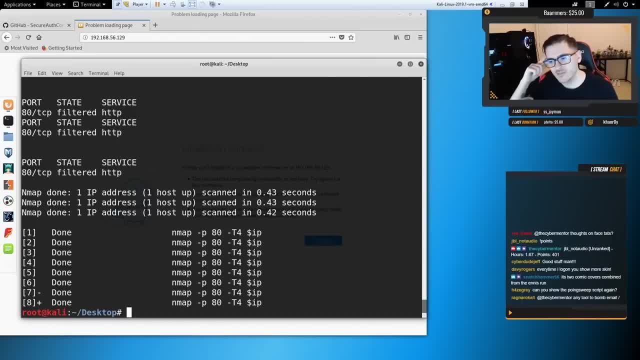 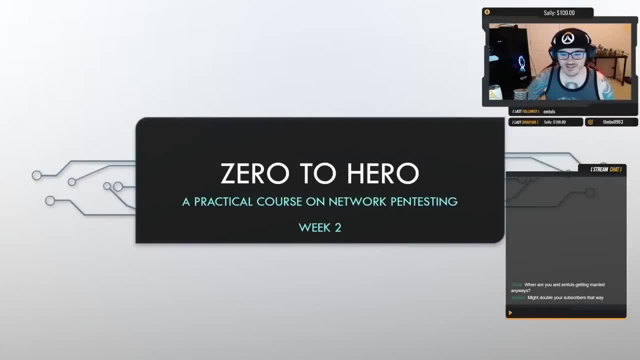 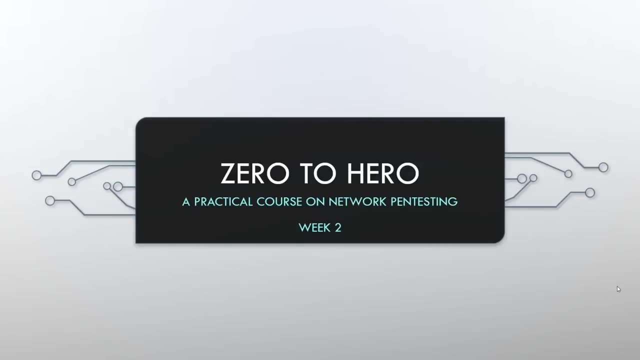 But these are the most frequent commands that I can think of that you're going to see in your career. All right, Let me just share this screen with you guys. Welcome to Zero, to Hero, Week 2.. So a few things. tonight We're going to be doing housekeeping. 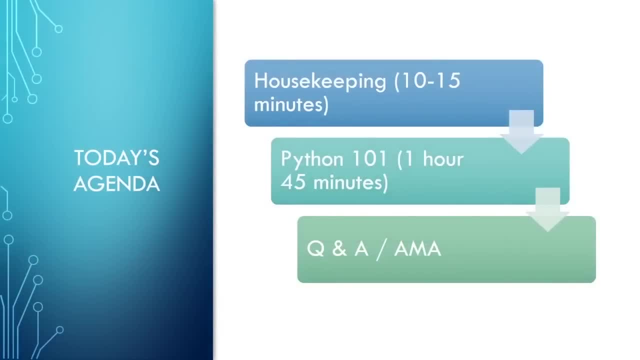 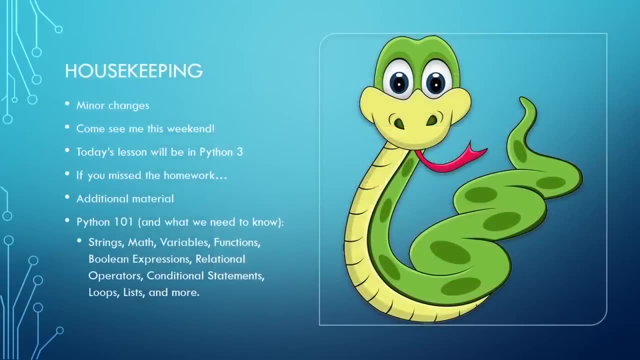 Maybe 10 minutes, 15 minutes. We're going to go into Python 101 for about an hour and 45 minutes And then we are going to do some Q&A, as always, So right into the housekeeping. So we made some minor changes. 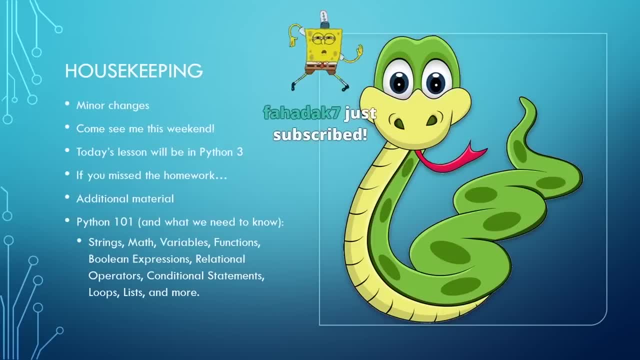 Had somebody do a little pen testing on my system, the gaming system that we have, the heist and everything else. They figured a way out to game the system a little bit, So I've taken that down temporarily. I brought it back up. 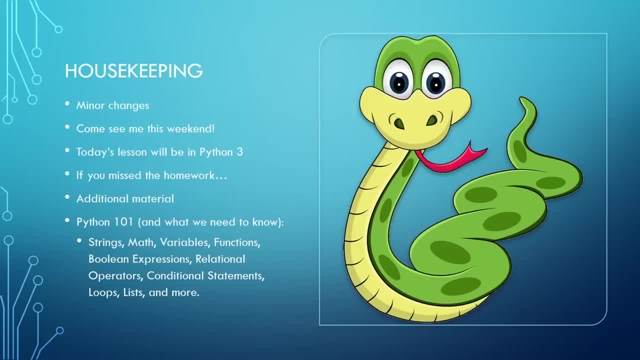 Just changed some of the rules on it. I let them keep their points. It was a vulnerability that I left up and they got the reward for the points. You'll notice that the heist system only allows you to play once every three minutes. 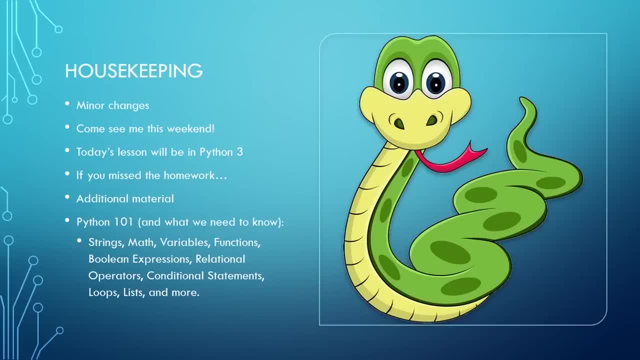 That is just because we received a couple complaints that it was just full of people typing and they couldn't keep up with the game channels. So games are there to have fun, win money, whatever You guys like gambling. Other than that, that's really it on the changes. 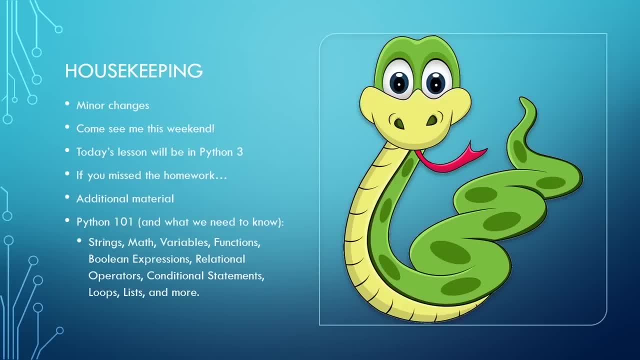 If you are in the South Carolina area this weekend, I will be at B-Sides on Saturday in Greenville, South Carolina. I will be on a panel. If you want to hang out, come see me. Just have a good time at B-Sides. 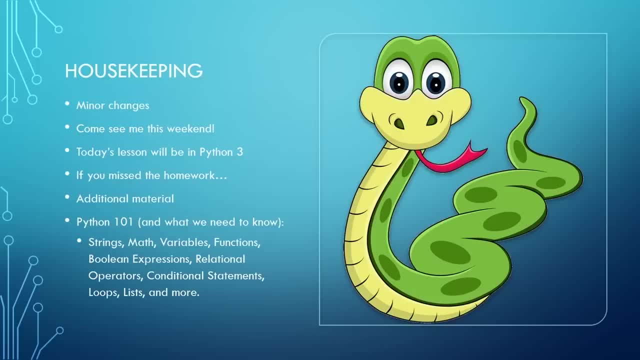 There's going to be a lot of cool stuff going on there this weekend, So please feel free to come say hi if you are there. Thanks for the sub as well, Fahad. I appreciate that. So today's lesson is going to be in Python 3.. 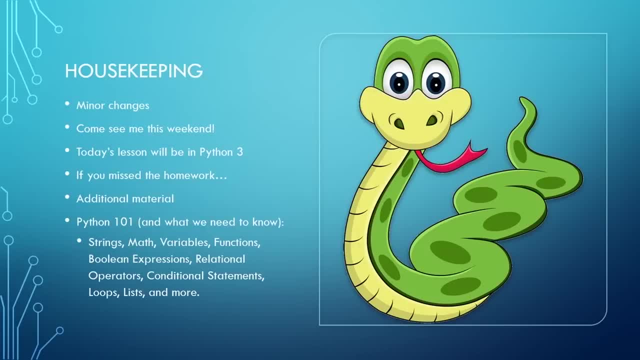 There are still some debates whether Python 2 or Python 3 is the right way to go. My reasoning for Python 3. is that we're ending support for Python 2 in 2020.. So the sooner that we convert over, the better, I think. 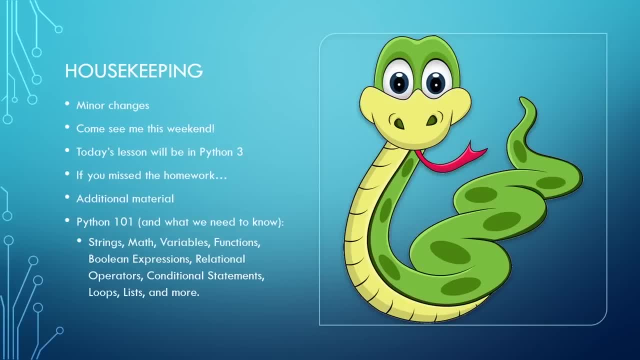 So I'll give you some resources and references that are Python 2. that you can work on converting into Python 3.. So if you missed the homework announcement, if you're not on the mailing list or in the channel, the Discord channel, then you probably missed what we did for homework over the week. 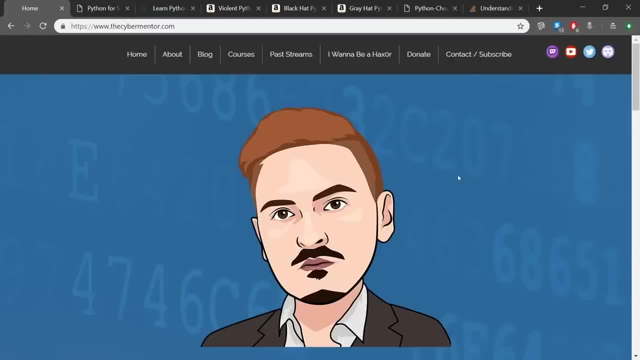 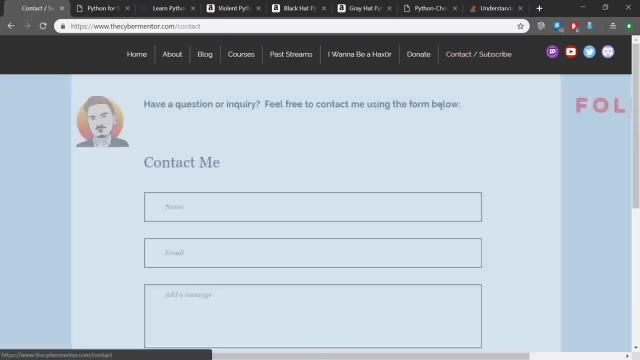 Let me go ahead and just pull that up for you guys. So if you are not already subscribed to the mailing list, if you come to thecybermentorcom and you just hit contact subscribe in here, you can just subscribe. That is where I send out the homework. 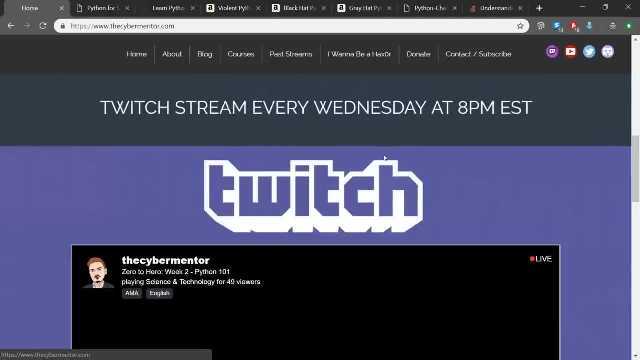 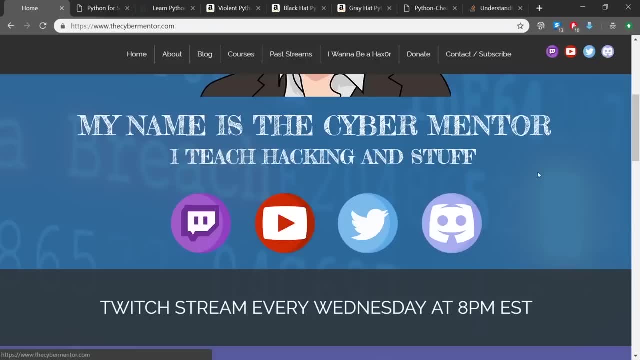 If you do not like email, I also paste the homework once a week inside of our Discord. If you come to this Discord link right here or up here or anywhere on the page, you can get that information. But for those of you who missed it and those of you who are following along at a later time, 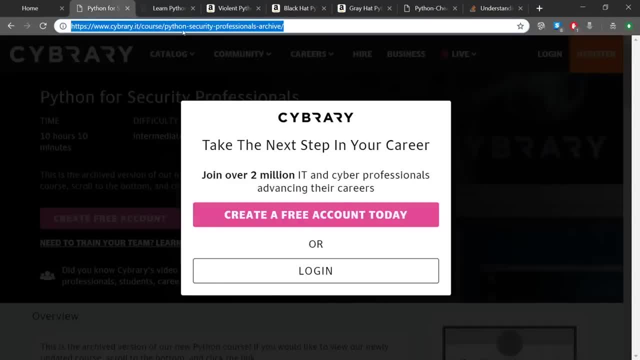 just watching the streams. we did cover Python Security Professionals Archive here. This is called Python for Security Professionals. It is by Joe Perry at Cybrary. He also has a course that is introductory Python. You may get those two confused, so make sure that you're looking at this one. 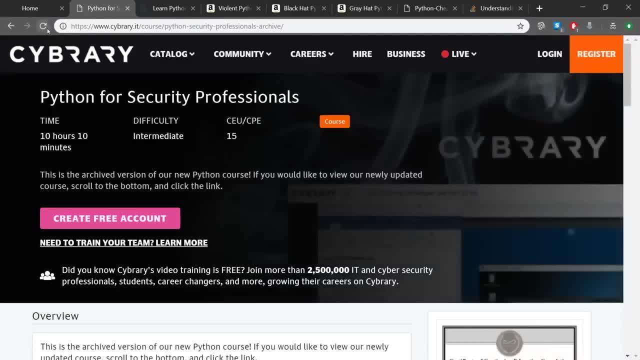 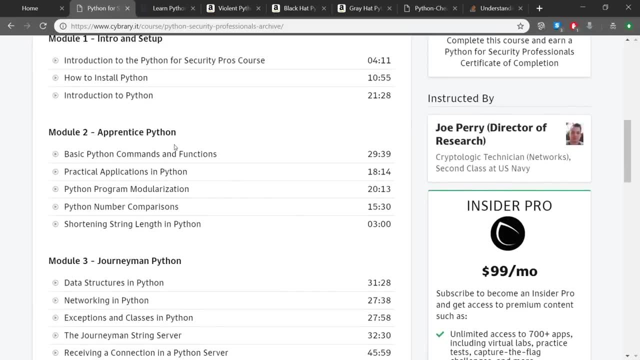 Let me refresh here. Hey, thanks for the subs again, guys. I appreciate that. So it has some nice buildup. I did this on my way to the OSCP. I did it like a week or two before the OSCP and it was plenty enough to get through the OSCP. 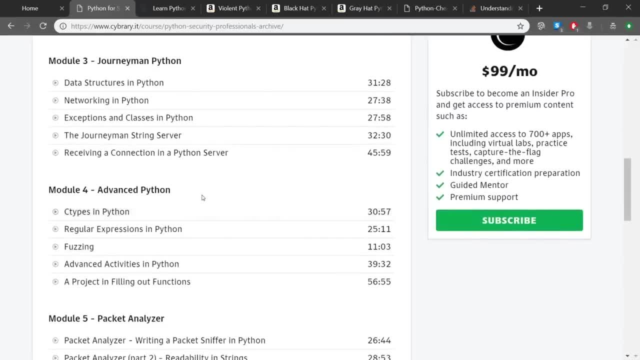 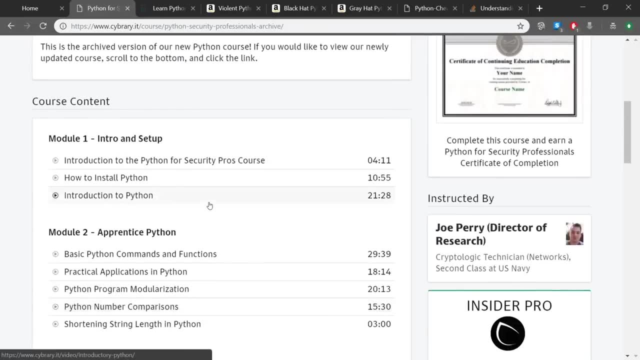 So it has Apprentice Journeyman Advanced. You end up building some cool projects out and it's one of the things I recommend. It is Python 2.. It is a little bit older, but it doesn't mean that you can't learn the concepts. 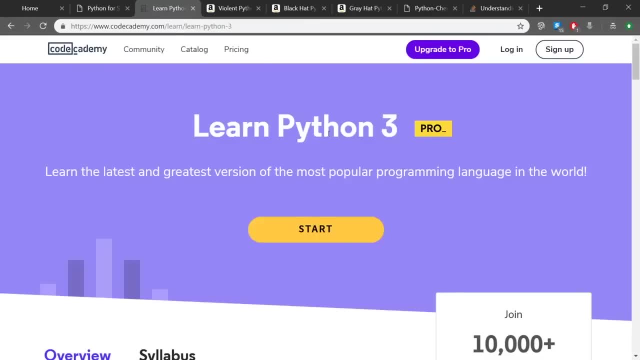 and that's really what we're after today. The other one is Learn Python 3 over at Codecademy. So Codecademy gives you a week free of pro. You don't have to enter a credit card, nothing fancy there, It just gives you a week to try anything out that you want. 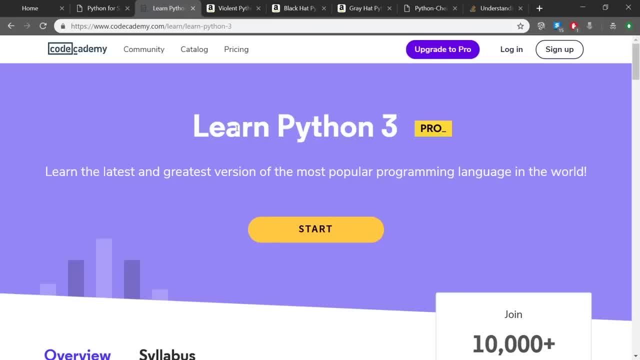 So if you register under a new email, if you've already used it or whatever, you can come in here and learn Python 3 for free. So this is also a great resource if you want to get some hands-on. There's plenty of other ones. 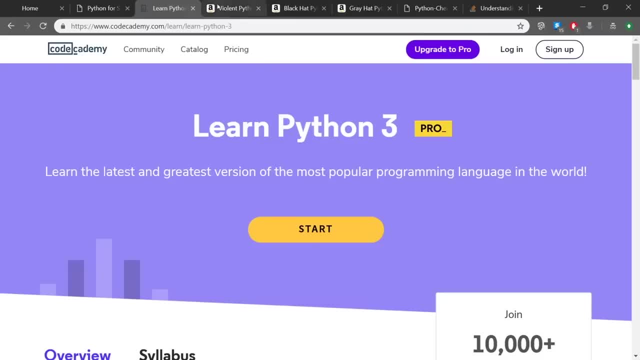 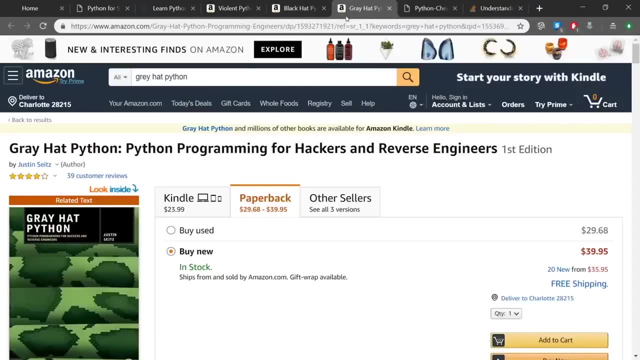 If we want to talk about resources that are hacking-related, we've got the well-known Violent Python, we've got Black Hat Python and we've got Gray Hat Python. So great books. All of them are a little bit older. They're written in Python 2.. 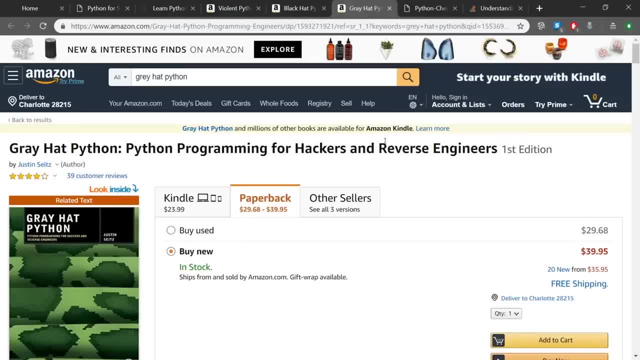 So my challenge to people is to try to take some of the concepts that are in these books and try to convert them over to Python 3.. Not only is that a good challenge- you know, just for yourself- but it really gets you to understand the concepts on both the Python 2 and Python 3 level. 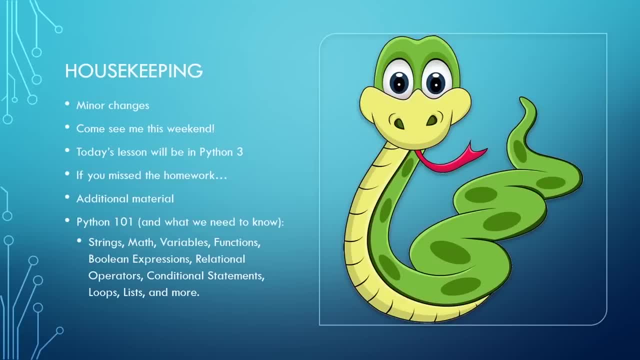 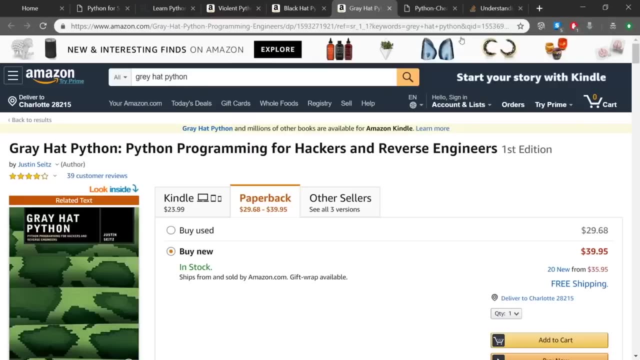 So, other than that, let's go back to our PowerPoint real quick. I do have additional material Other than what I just gave out. I have a cheat sheet. Let me paste that into the chat. This is provided by Jeff. Jeff is one of the students and this is great. 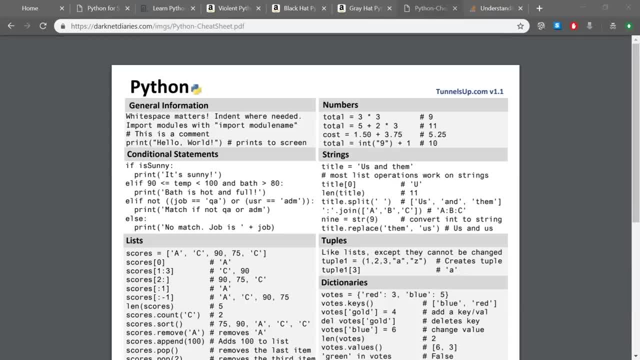 This is hosted over at Darknet. If you don't know what Darknet Diaries is, I'd recommend checking that out too. It's a really great podcast, But this is a nice little Python cheat sheet that, if you want to remember anything from tonight. 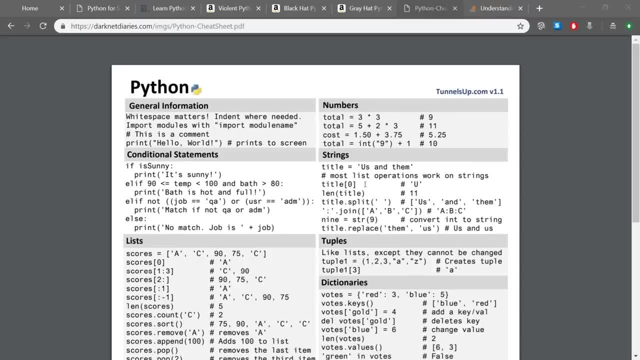 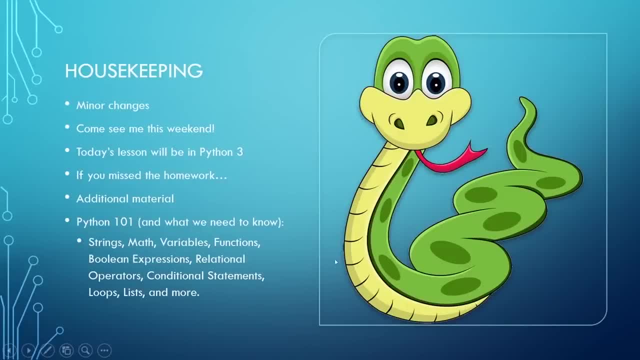 has just really well laid out. This is beginner stuff. This isn't all the things you're going to need to know, but we're going to talk on that as well. So, when it comes to Python 101 and what we need to know, 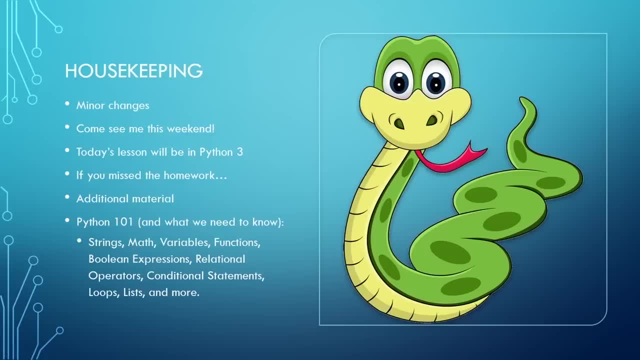 I have about an hour and 45 minutes. It's kind of what we allocated tonight that I want to teach you guys. That's obviously not going to be enough to teach you everything you would ever need to know in Python. You would need weeks and weeks of that. 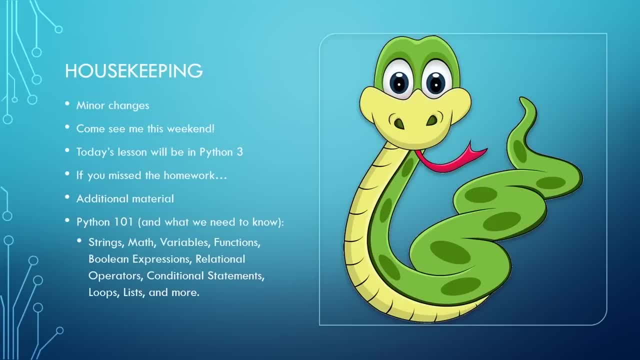 My goal for tonight is that I want you to be able to understand what you're looking at and reinforce some of the concepts from last week, Because last week we talked about scripting, We covered loops, We covered variables, We saw some scripting concepts. 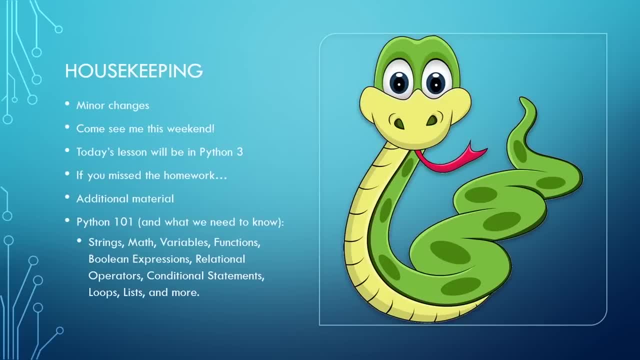 We're going to reinforce those harder tonight And by the end of it, my goal is. I'm going to take two scripts. I'm going to show you two scripts. They're going to be advanced. They're going to be more advanced than what we've covered. 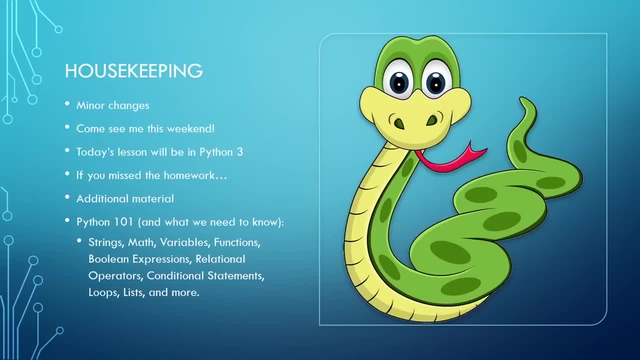 One's going to be on the medium, basic side. The second one's going to be on the more advanced side. We have not covered half of what's in there, But my goal is that we read it and you can understand what's going on. 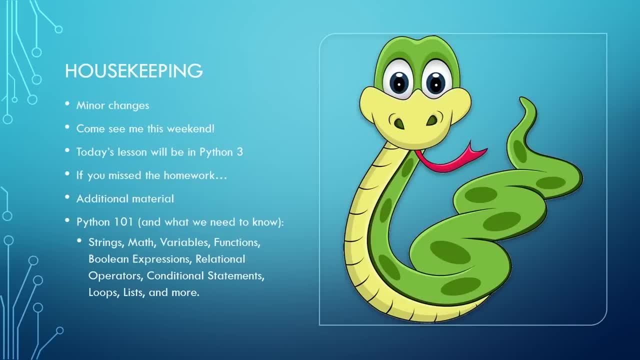 And at a Python 101 level. really, that's what we need At a junior pen tester level. you just need to understand what's going on As you move up and you get more advanced if you want to start writing your own scripts to automate things. 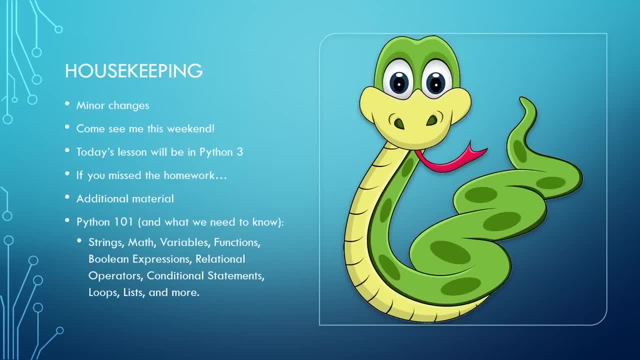 if you want to get better at this, that's your priority. It helps you absolutely. The better dev you are, the better coder you are, the better hacker you can be, I think. in my opinion, It does not mean that you need to know Python full in and out. 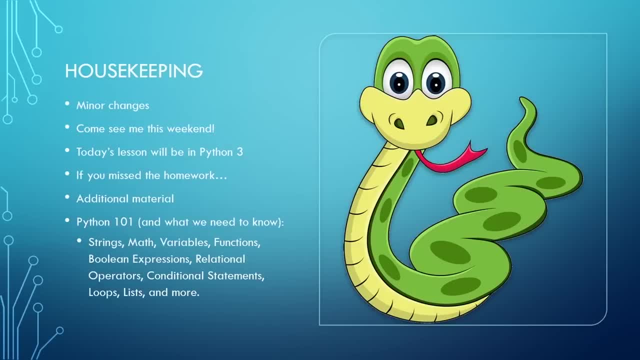 You can make a career out of pen testing without ever knowing Python fully. Just being able to understand what you're seeing really, really helps. So if, at the end of the night, I'm going to put up a poll If you feel like you could use another week of Python, you want more of this. 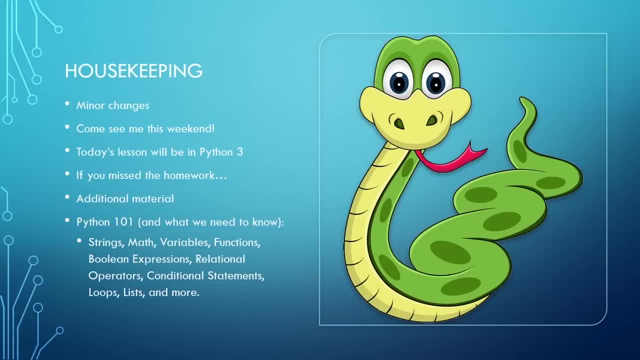 we'll dive into it next week again, Maybe an hour, maybe the whole week, depending on the lesson plan that I put together. If you feel like, okay, we're good, let's go on. this is fine. you've provided homework that covers more than this. 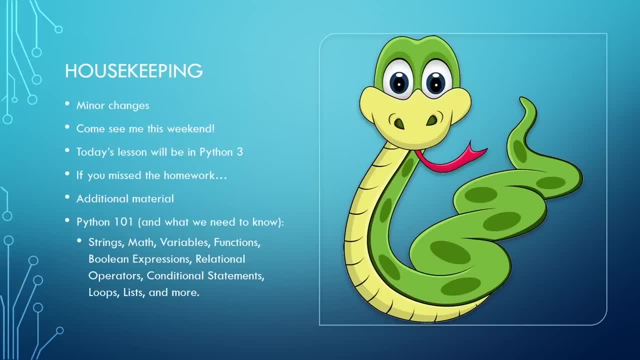 I want to move on to the hacking. then next week we're going to actually start into the hacking concepts and start with a little reconnaissance and have some fun. So it's completely up to you guys. When the night is over, you'll decide what we do next week. 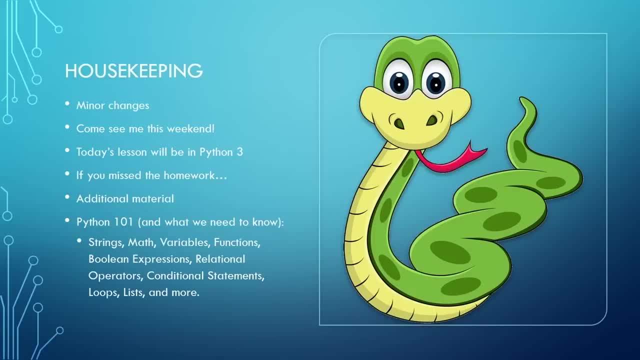 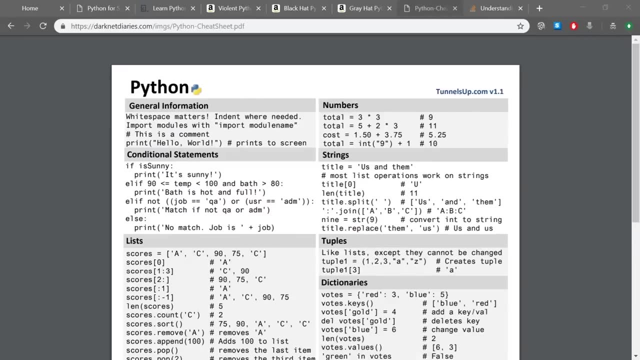 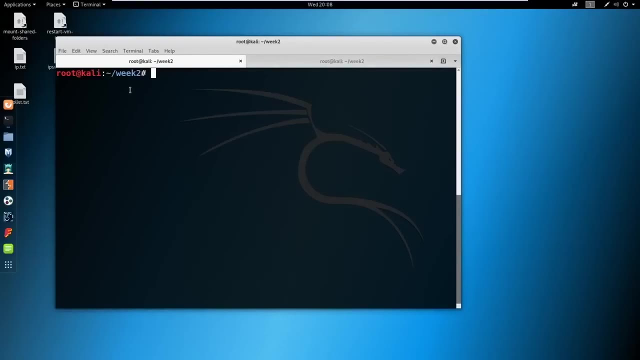 So, other than that, we're going to go ahead and just dive right in. So I'm going to be using Kali tonight, Same as always, And what I've done is I've made a folder here, just made a directory called week two. 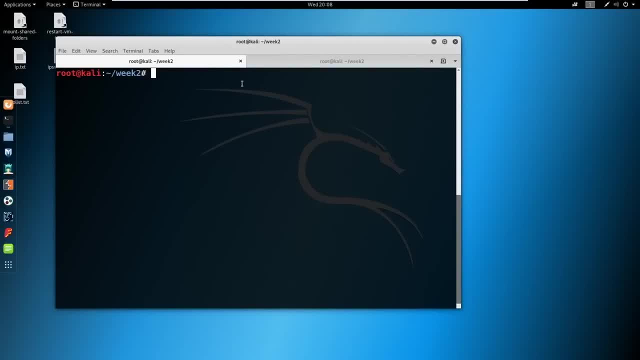 I just recommend that for keeping all of your information in here. What we're going to be doing tonight is making one long Python script, So it's going to be a little jumbled. We're going to make comments and stuff to really make it kind of make sense. 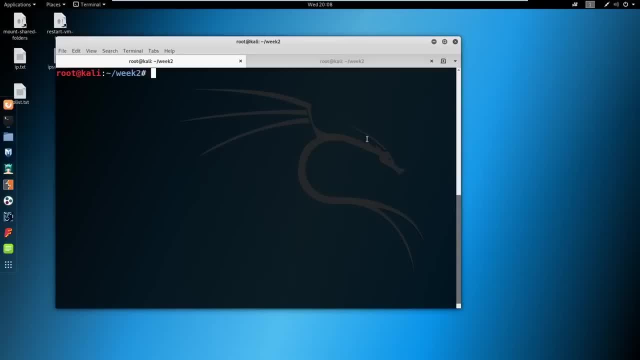 My reasoning for this is I want you to have everything that we did in one place, And so when you want to go back and reference something, you have a notebook kind of already started. You've got the concepts already there. If you want to build upon it, you're more than welcome. 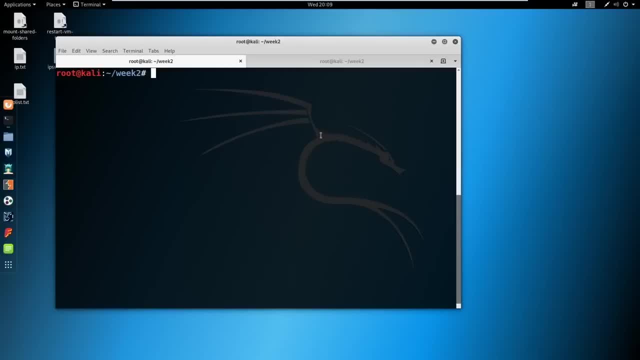 And we're going to extend from there. So let's go ahead and let's get started. So if you were having issues with gedit, like I was last week, if your gedit does not work when we do this, go ahead and just type in. 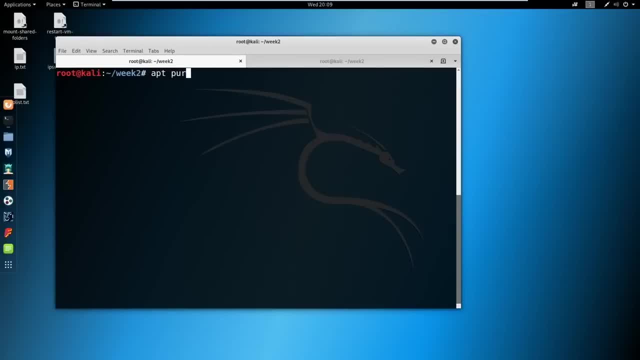 apt purge gedit and then apt install gedit. I'm going to be working in gedit today. We're not going to be working in IDE. If we cover next week, we'll cover IDEs and everything else, But for now gedit is going to be fine. 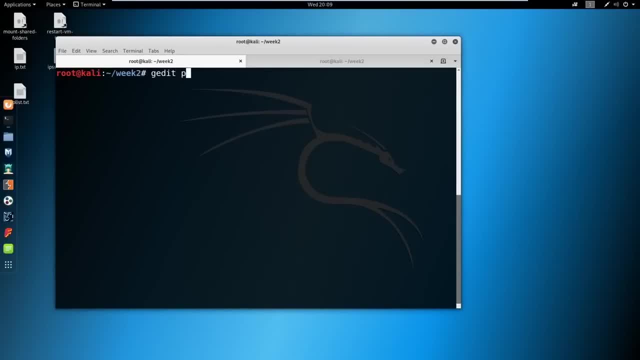 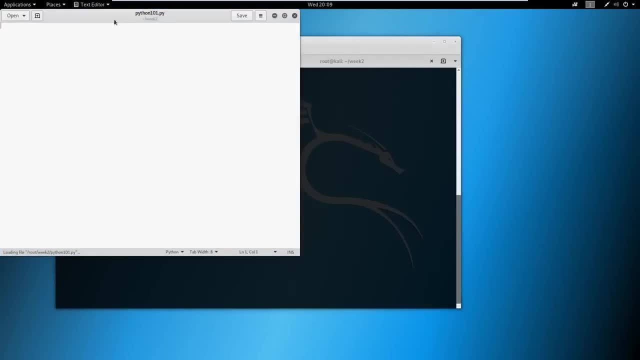 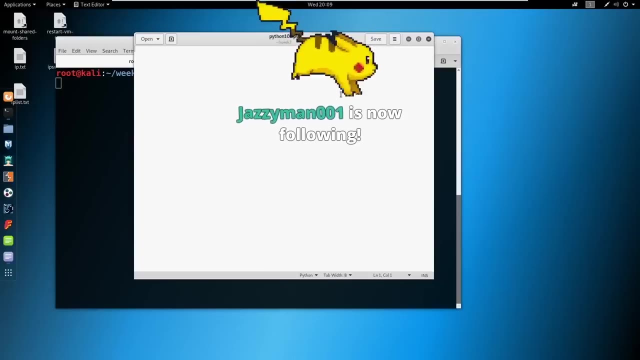 So I'm going to call this python101.py, Okay, And if this is too small, let me know, guys, and I'll increase the size on this. So what we're going to be doing is we need to first declare, like we did last week. 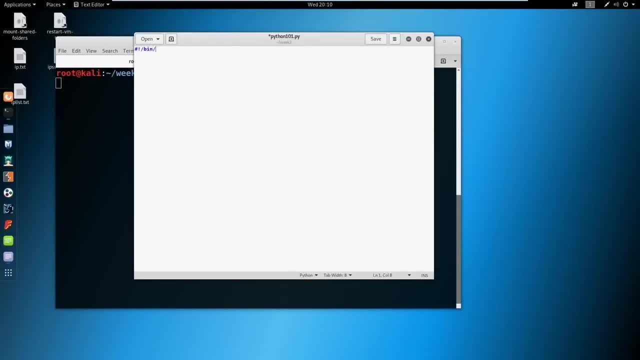 we're going to declare, with a hashbang of a bin, python3.. Remember, we did that with bash. So same thing here. We're just going to be calling out python3.. And the first thing I want to show you guys are strings. 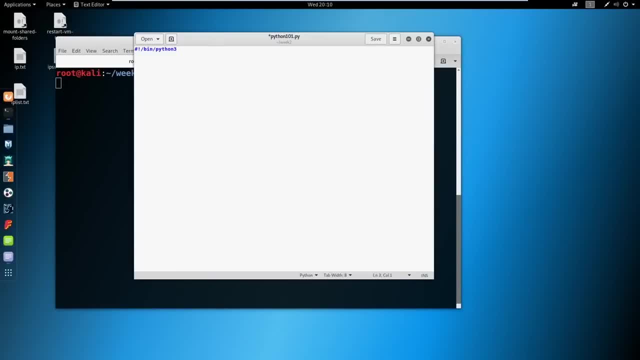 So you know the typical program starts. if you take a programming class, it always starts with hello world. So it's not going to really be any different here. What we're going to do is I'm going to put in a comment first. 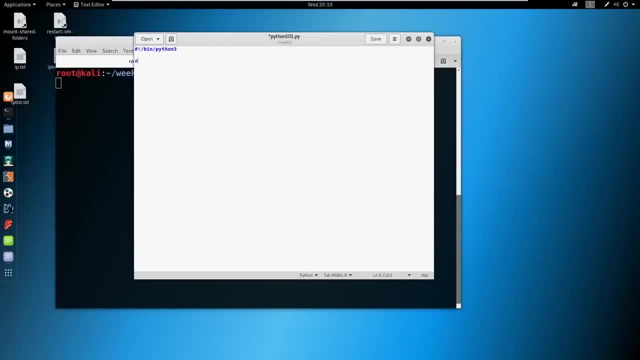 And this is just a comment- when you use a hashtag like this, I'm just going to say this is how you print a string, or we're going to be printing a string And we're going to be using the print command to go ahead and print out to our console or our terminal here. 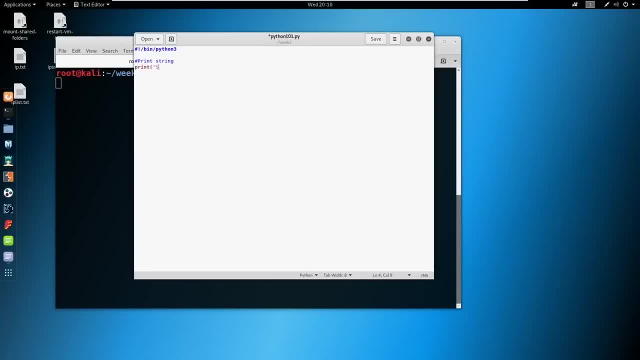 So we're just going to say print And we're going to call this little category strings and things. Now you've noticed that I've put everything here in quotation marks, So if you see something in quotations like this, this indicates that it's a string. 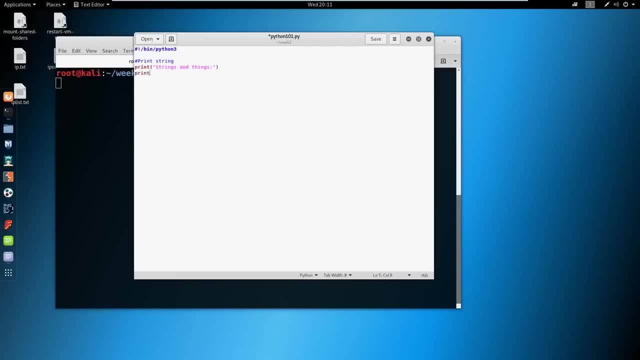 Now, alternatively, we can do that with single quotes. We can say hello world, like this, And that'll be fine as well. And finally, we can also print something like multiline. We can say: hello, This is a multiline string And we'll just put it in triple quotes, like that. 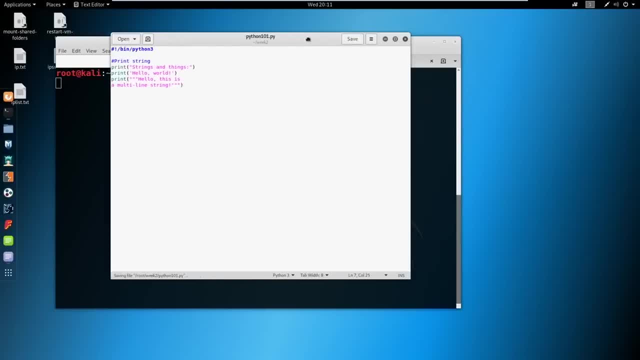 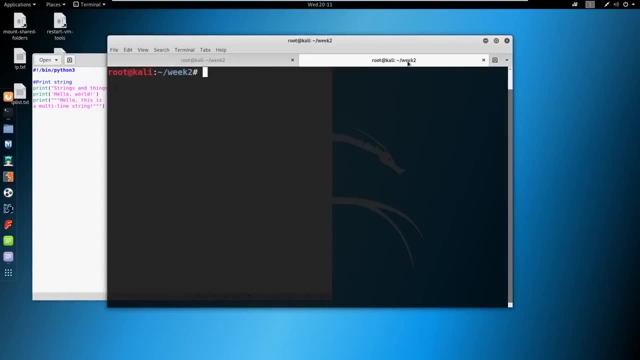 So let's go ahead and just save this And what I've done, so we don't have to keep closing the editor out. I've gone ahead and opened up a new tab right here that we're going to just be firing off this script. 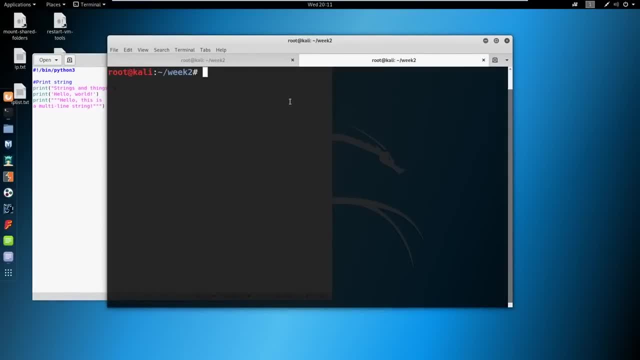 and saying hello world, And we're seeing what posts to the console. So what we need to do first- remember from last week- we need to make this file executable. So, whatever you called it- python101.py- we're going to make executable. 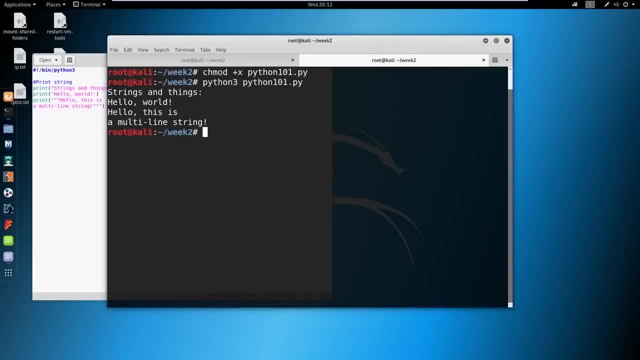 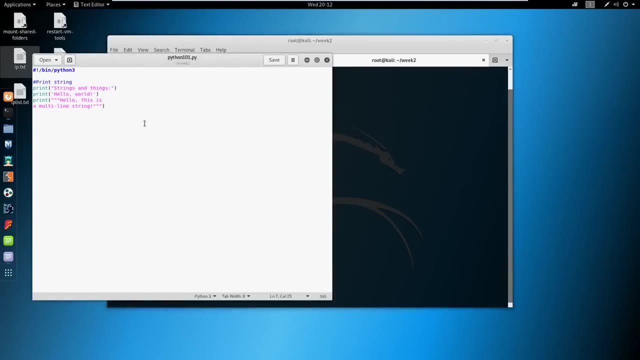 And then I'm just going to say python3, python101.py. You can see we've pasted out strings and things. Hello world, and then hello, this is a multiline string. So everything is working out so far And we can also do concatenation inside of print if we wanted to. 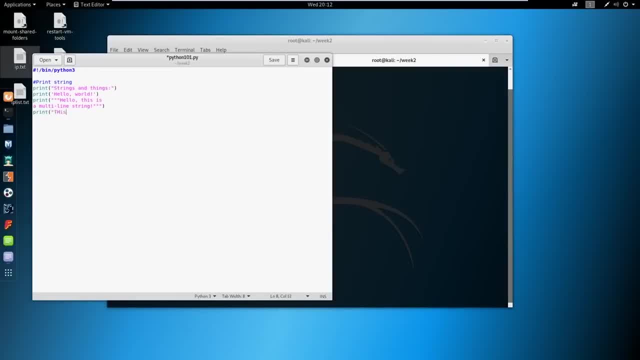 So if we said print this is, and then we can just put plus in here and say a string, That would also work. We'll get more into concatenation a little bit later. Okay, so what we're going to do and kind of separate this from our sections. 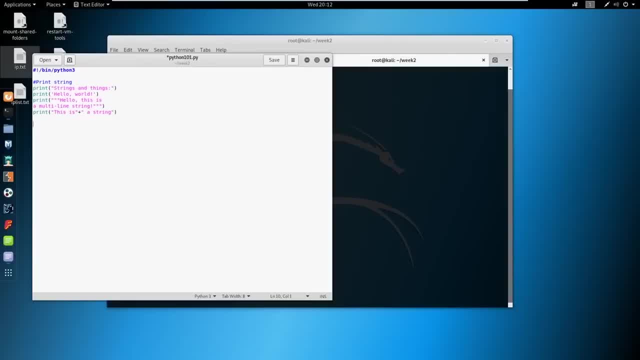 this is just a brief introduction here on strings. What we're going to do is just print a new line. So I'm going to show you how to print a new line And then we can put a comment right here to say a new line. 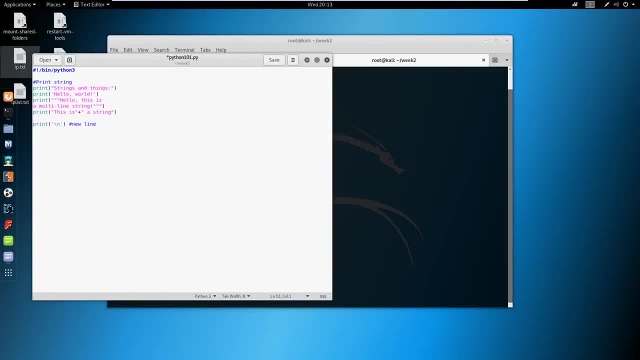 Okay, And then we're going to dive right into math, And if you guys need any concepts slowed down, please let me know. We've got a lot to cover tonight, So I'm just going to dive through some of these ones faster. 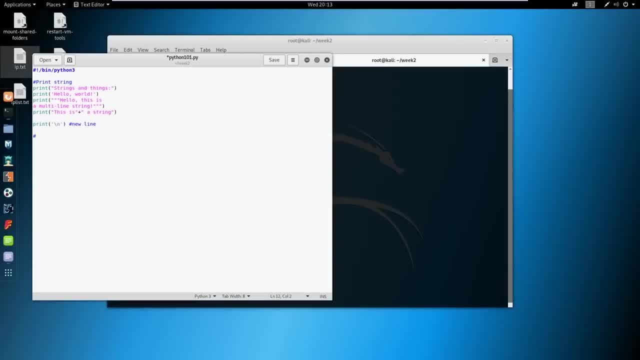 Some of the other ones that we're going to go through are going to be slower. So, hey, Gray, how's it going? Okay, so for math, we're going to print out. We're just going to call this one math time, right? 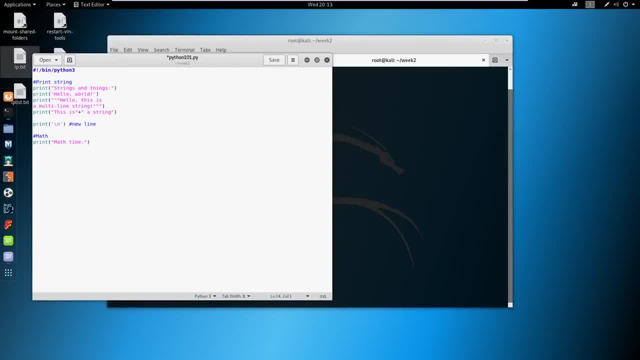 So that's our little section here, And we could do a lot of math in Python. We could do a lot of math in Python without having to call any sort of math module, So let's take a look at some of the things that we can actually do. 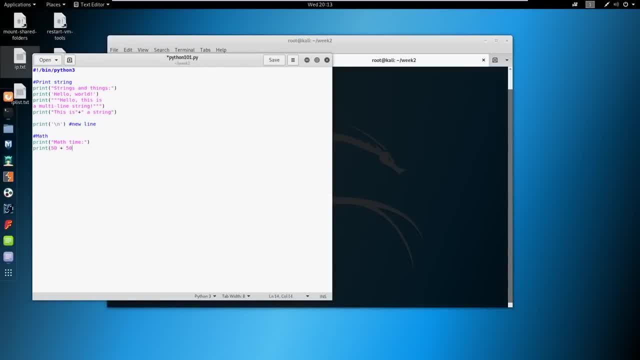 So we can add And you can use whatever numbers you want. I'm going to go 50 plus 50.. I'll put a note next to it that says add: We can subtract 50 minus 50.. We can multiply 50 times 50.. 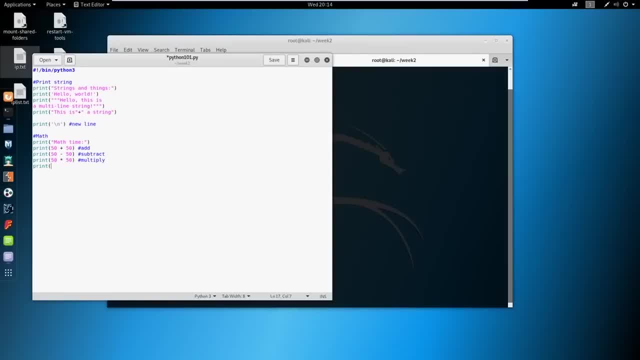 We can divide, And we'll talk a little bit about division here in a second. We can do some crazy stuff, right? We can do 50 plus 50 minus 50.. 50 times 50 divided by 50. We'll just call that PEMDAS. 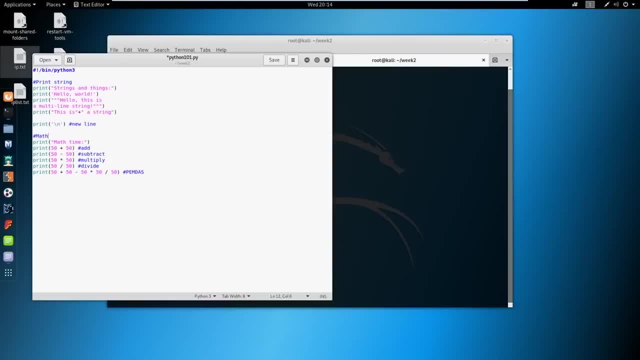 Is it maths? All right, we're doing maths Here, Leah, there you go, Maths. And then we'll say: print 50 times 50.. Or 50 times 2, sorry, We could do exponents, So we're raising this to the second power here. 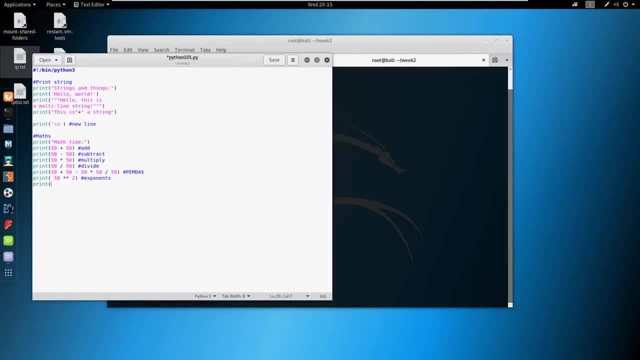 A couple more things and I'll cover what all these are. again, I have a space in here. Spacing is everything. Don't have the spaces. We could do this little modulo here, So this is called a modulo, And we can also do something that looks like this: 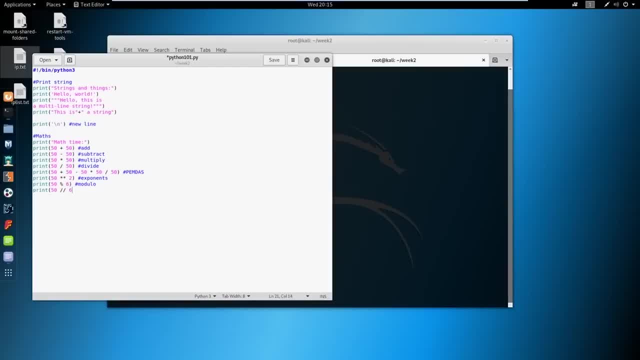 We'll just call this a number without leftovers, Okay, So for a couple of these things. So this is going to multiply 50 times 50 because we're doing exponents, right? That should make sense. If you're not, math background, that's fine. 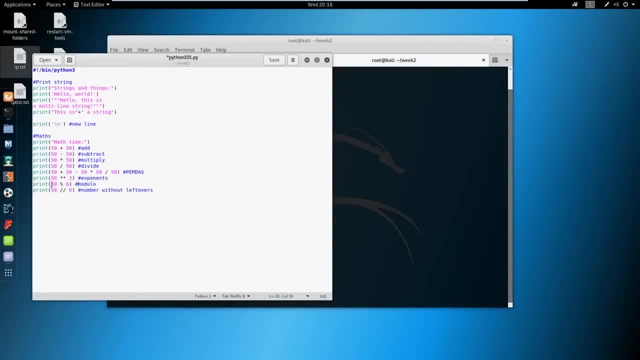 This modulo here. What this is going to do is it's going to take whatever is remaining. So 6 times 8 is 48. So this should return 2, because 6 goes into 50 eight times and then has 2 left over. 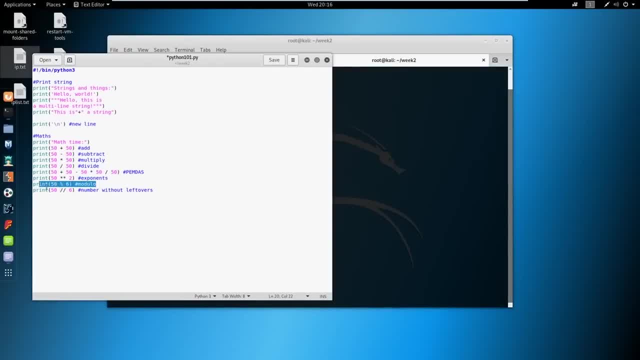 So for some reason we wanted to do the remainder. That's called a modulo. We'll do that When we divide over here 50 by 50, if it was 51 by 50, it would return one point, whatever right. 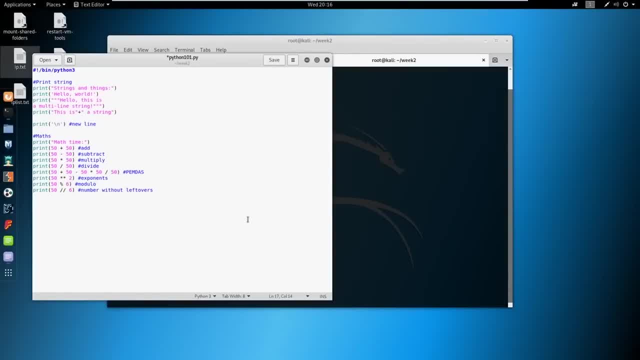 So we would have leftovers, We would have a non-int, We'd call that a float. But here, if we wanted a number, just a number with no leftovers after it, no digits or anything, here we would use this double division. 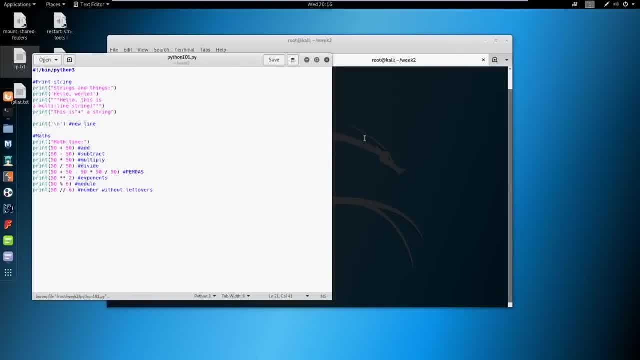 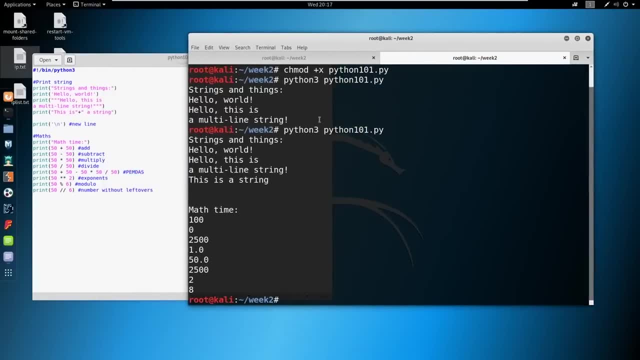 And we can kind of take a look at what all this looks like. So let's save that And let's just tab up and print again And you can kind of see what this looks like. So if we don't have a decimal place here, 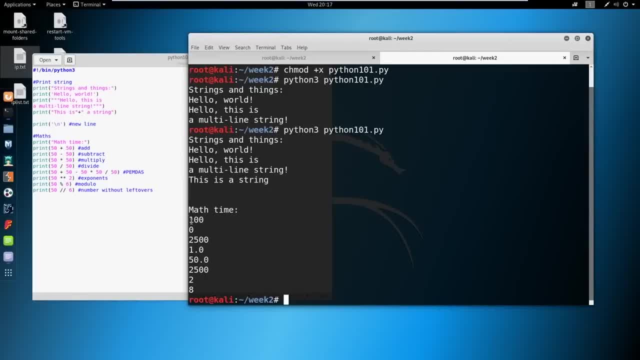 then we can assume that the number is actually just an integer. But when we do have the decimal, that is called a float, And we're going to talk about that in just a second. Those become important when we want to declare our numbers. 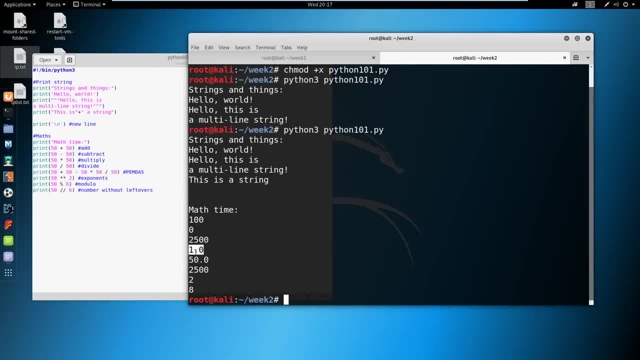 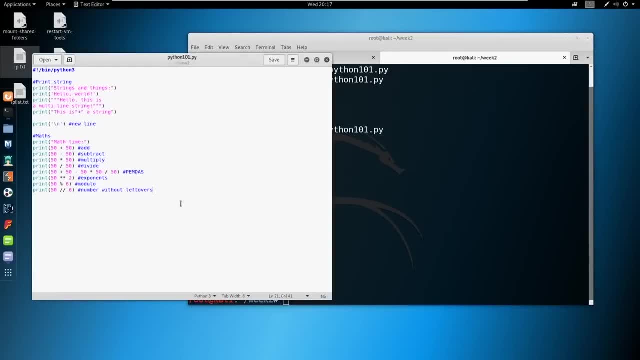 In Python. these are two different things. So we've got to make sure that we know exactly what kind of number we want, And we'll get into that just in a little bit. So on top of strings and maths, we can do some cool other things as well. 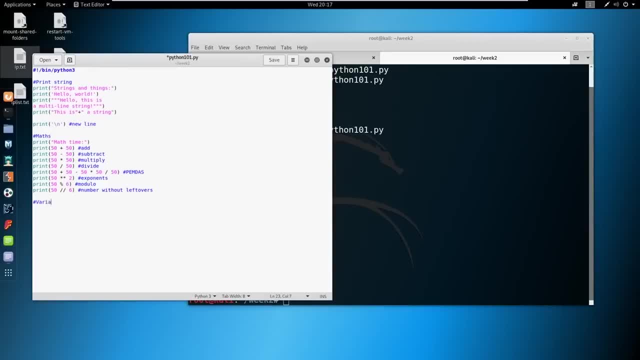 Like, we can declare variables. So let's create a section here and we'll just call it variables. We'll call it methods as well, because we're going to have some methods. Hey Nate, how's it going? man, I'm just going to capture this new line, copy this new line. 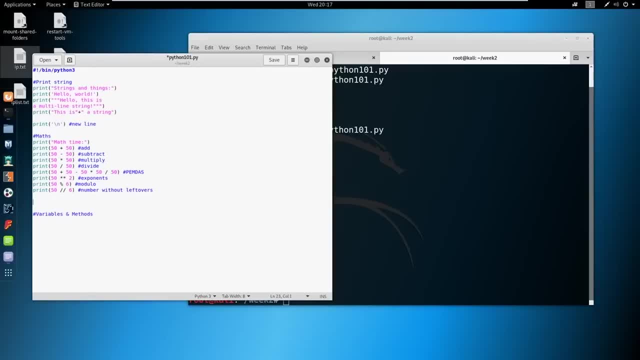 and we're going to paste it right in here. How long will it take somebody with no programming background to be comfortable with Python? To be comfortable, it depends on your own level, But it's pretty basic. They're moving towards Python for the introductory programming classes now. 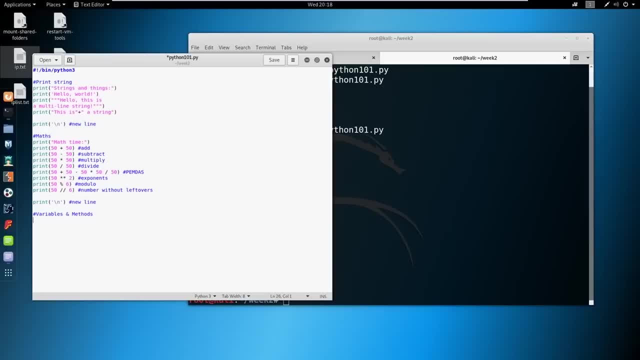 Like the 101s, are starting to do Python instead. A lot of the concepts are really basic. I think to get an intermediate level you'd probably have to spend some time in it, But at an introductory level I would say a month or two of just playing around reading it. 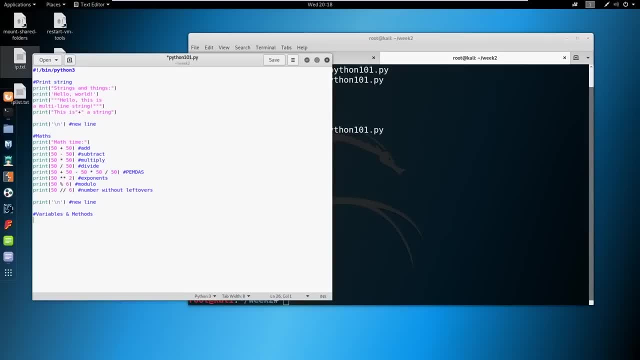 It doesn't take too long. It's not basic enough where you're going to become a developer overnight, but it's definitely probably the most simple, or one of the most simple programming languages to learn. That's why it's considered a decent foundation. 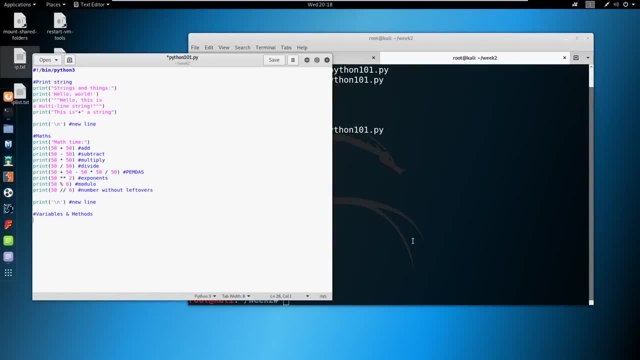 Okay, so we're going to have some fun with variables and methods. So, like we've been doing, let's just print a little title out, We'll call it Python, We'll call this fun with variables and methods, And let's declare a variable. 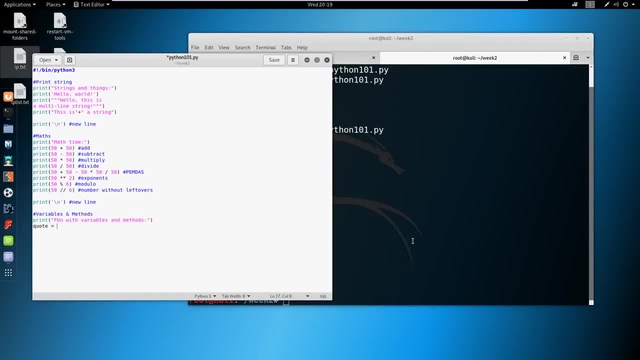 We're just going to call it quote And inside this quote we're going to have a string. So we're going to say thank you. I have some issues with my. I'm a caps lock person, not a shift person. 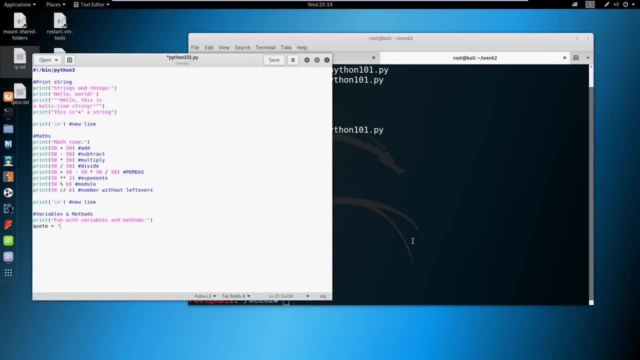 So the caps lock hang over when I'm typing sometimes and in my VM it hangs over just a bit. So we're going to say: all is fair and love and war. Don't judge me, guys. Don't judge me. I could type faster than probably most of you. 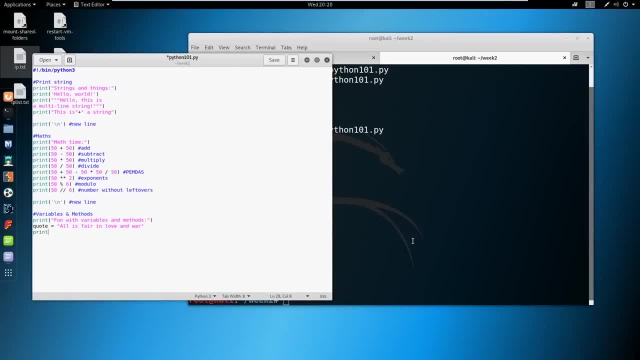 I won't say all of you because I am not going to claim that. Okay, So we say print length quote here. So if we have this quote and we want to print the length of the quote here, we could do that with just print length and the variable quote put into it. 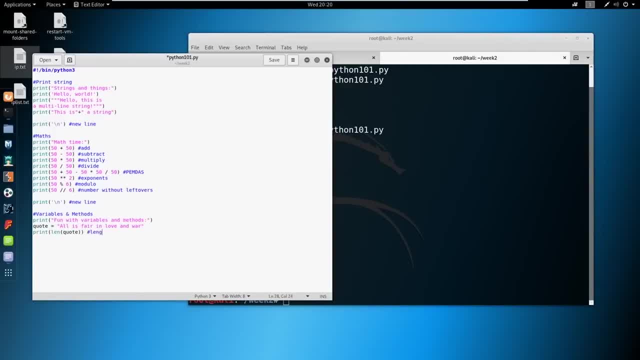 And I'll just say length. You'll see what all this looks like here in a second. And then let's say we wanted to turn that quote into an upper. We could say something like quote dot upper. This would turn it all uppercase, right. 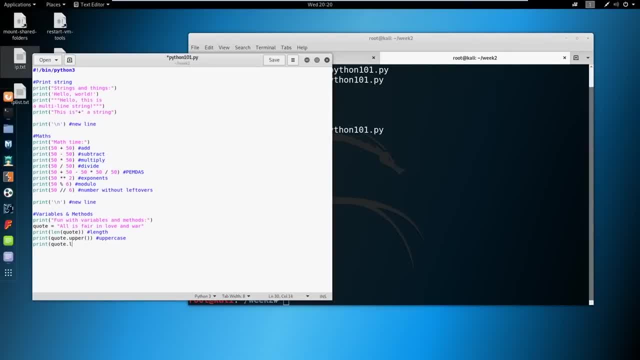 We can also do a lowercase. We could say quote dot lower, Make it lowercase. Or we can print it out in title form And let's see what that looks like. Oh, we've got caps lock squad in here. Yeah, guys. 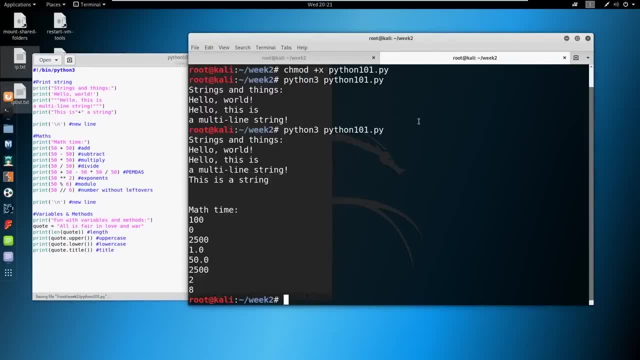 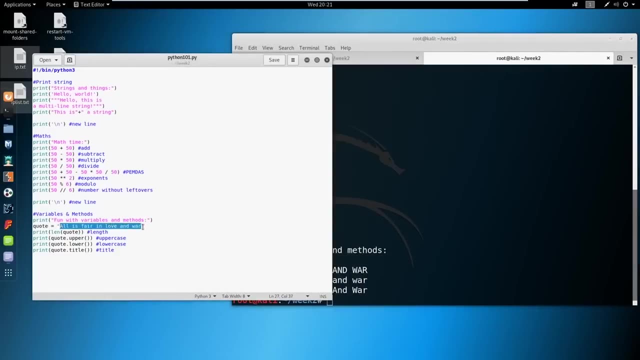 Back down. You don't know what's up. We rolled deeper than you think, So let's save this and run it again. Okay, So you can see it counted here with the length. It's got 27 on this string. All is fair and love and war. 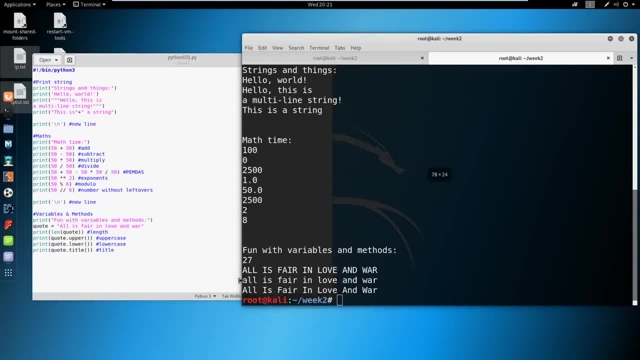 You can see it put it all in caps, All in lowercase, And then it titled it here for us as well, which capitalizes every first letter. It's not perfect, It's not like the official titling system, But if you need every first letter capitalized for some reason, you might be able to use it. 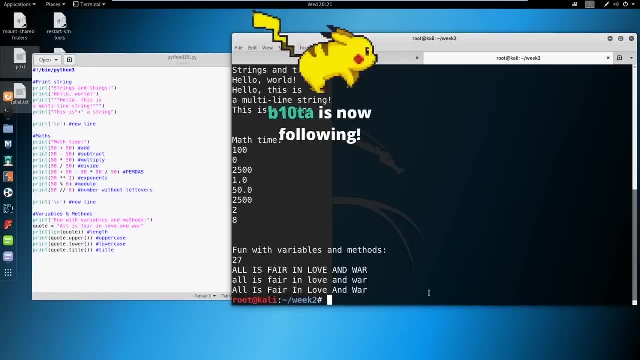 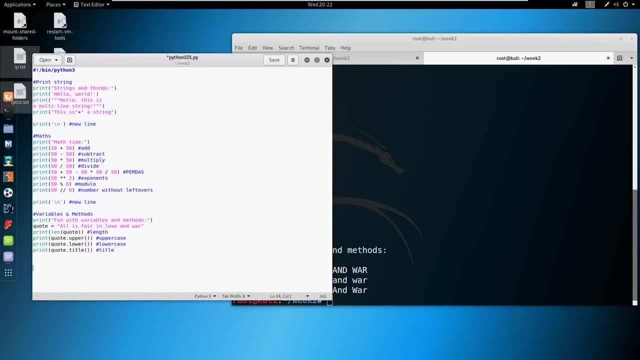 I don't know when you would use title. That's a great question. I have no idea. I've never used title, But it's a cool little thing to know. All right, Let's do another variable. Let's set your name as a variable here. 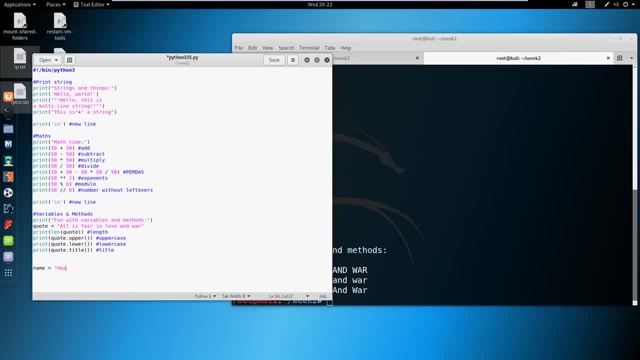 So we'll just say heath And then we'll say age: Okay, I'm 29.. Remember, this is an integer Right. It also can look like this: Int of 29.. If we wanted to declare it as an integer int of 29.. 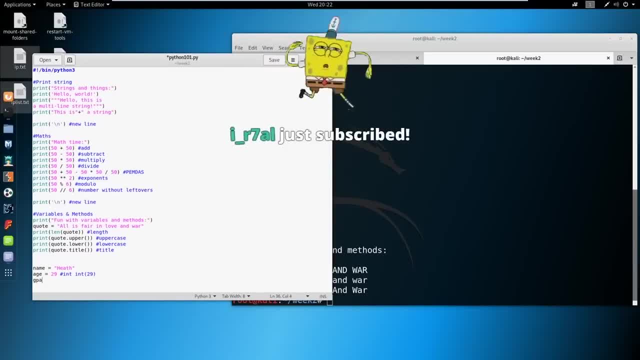 Okay, Let's say that my grade point average in college was a 3.7.. Now, why are we doing this? Because this is a float, Or it could look something like this: Float 3.7.. Hey, thanks, Shu, for the subs man. 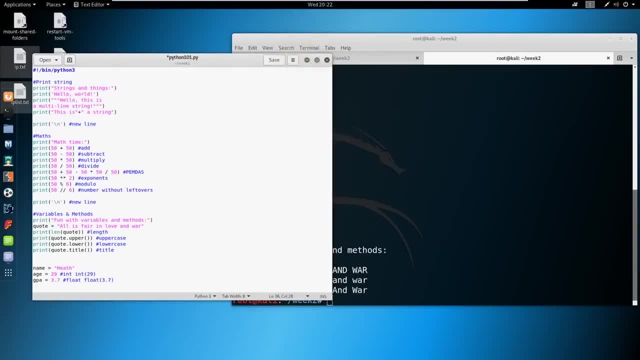 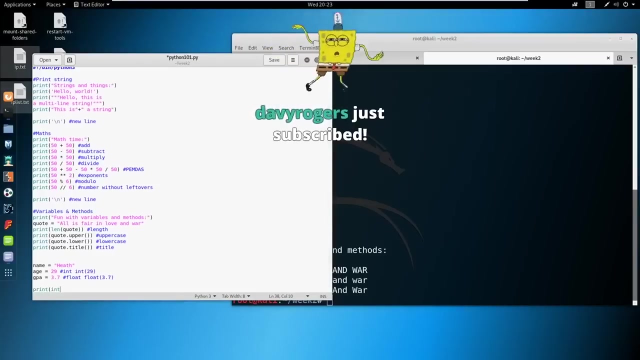 I appreciate that. You're awesome. Okay, So we've got these three here, Right? We've got three different variables we've got set. Now we can go ahead and print some things. Let's just say: let's print the integer of my age. 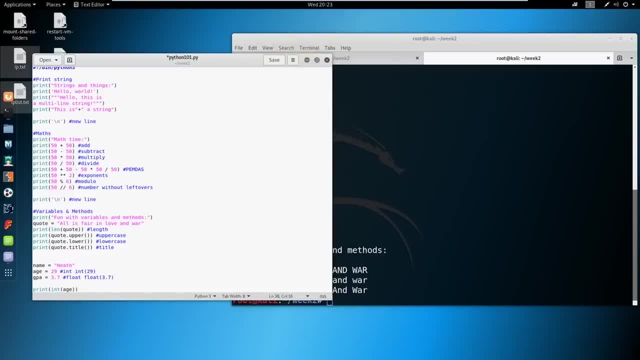 Right, That should return 29, because that's the int. But if we print the integer of my age, say I'm 29.9 years old, Right, If we print that out, what is that going to return? Let's take a look at it. 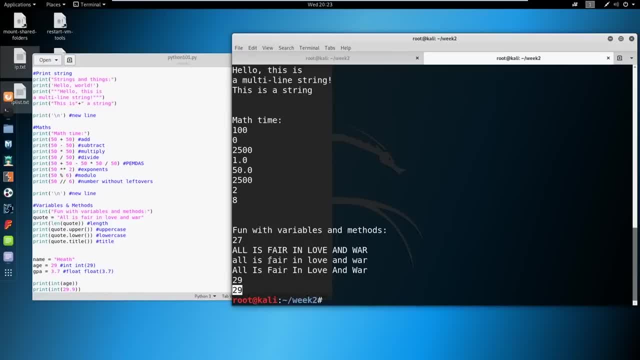 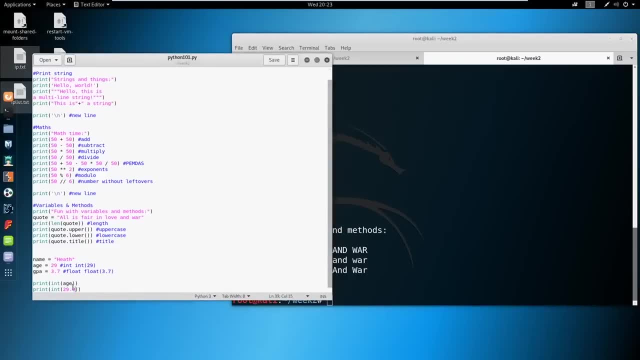 Up one, It's actually going to return 29.. So you think here that it would round up, but integer does not round. It just takes the first number and leaves off the rest after the decimal. So just keep that in mind going forward as well. 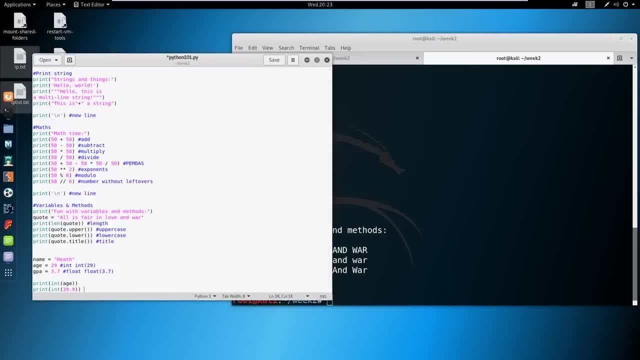 We can say a little note next to it Just say: does not round Right. We can also call out in a print statement. We can call out our variables. So if you want to say print, my name is, make sure to add a space. 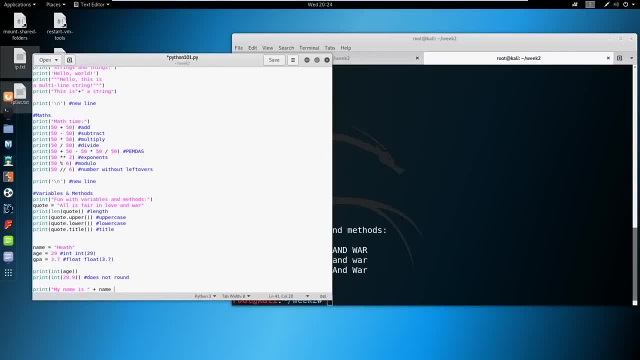 And then say plus name And then you could say space and I am space. Now we could say age and say years old. Now this statement is not going to work. Does anybody know why this isn't going to work? There's something here that is not like the rest. 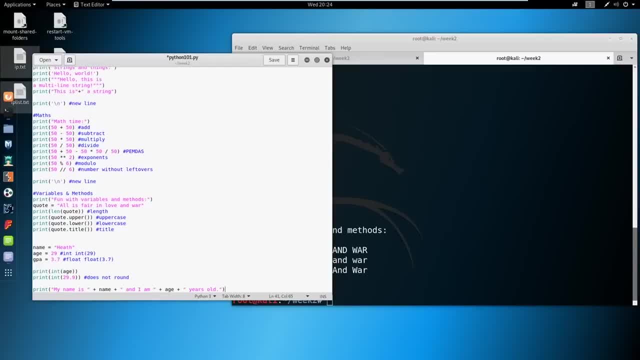 You have to convert to a string, Exactly String versus int. Good job, guys. You don't even need this lesson. You guys are too good. All right, So our age is sitting here and it's an integer. We can't put an integer in a string. 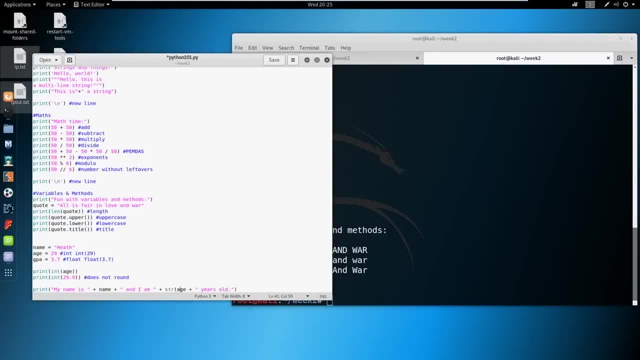 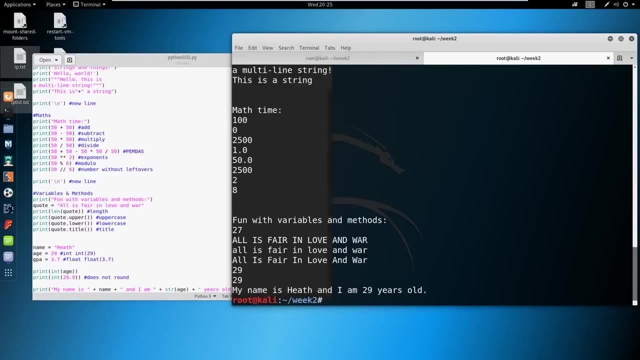 We're going to have to actually convert this to a string. We'll just say string. You cannot have different types. Exactly So we can see what this looks like. My name is Heath and I am 29 years old- Cool, So a few other things we can do. 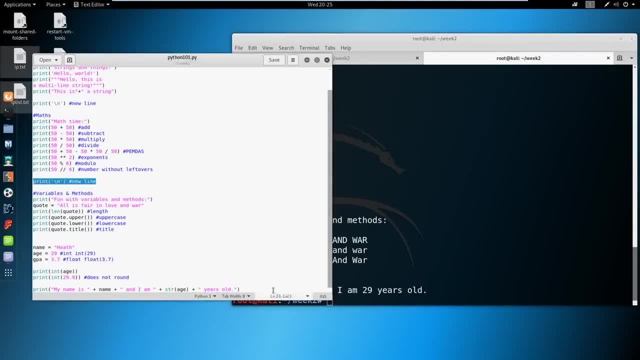 I'm going to go ahead and just add in a little new line here, Okay, So some things that we can use to play around with here. So let's say we have age and let's say that I got a little bit older. I can say that I got older a year. 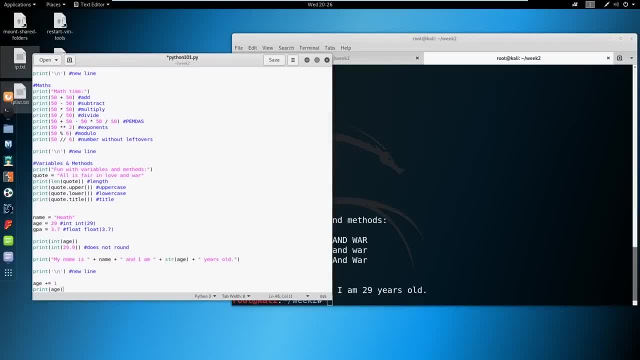 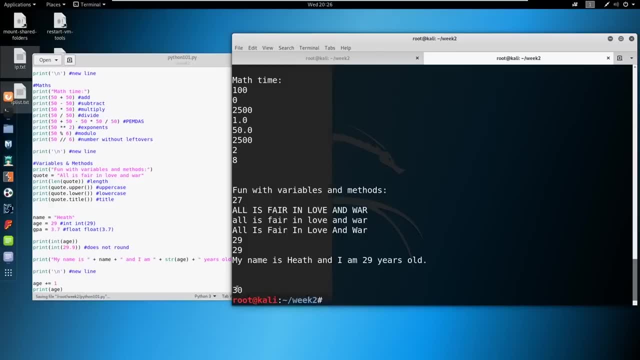 And if we printed this age, that would now make me 30. We can prove that by a quick save and run. Okay, So let's say I'm 30. So two things that we're noticing here. One is the obvious, right. 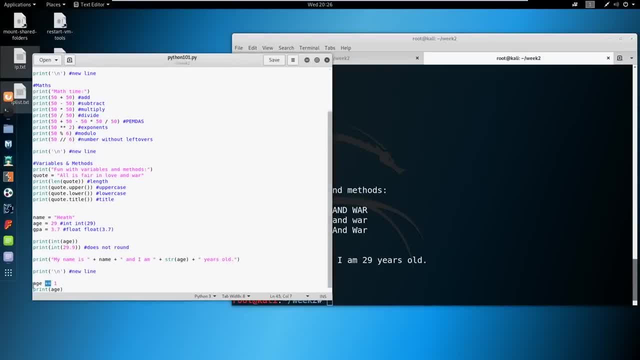 With the plus equals. we're adding something into what's already there, So we are adding a 1 into this age. Now I am 30.. Also, that means we are changing the variable itself, Right? So we are going to be changing the variable. 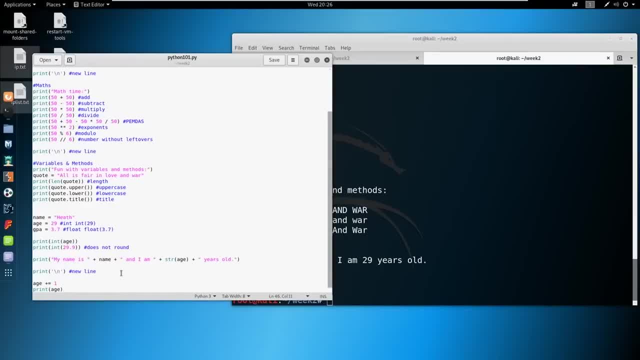 It's no longer 29. It does not always hold true 29.. Now it's holding to 30. So we've appended the variable. So we could also do, though, something like: birthday is equal to 1. And you could say: age plus equals birthday. 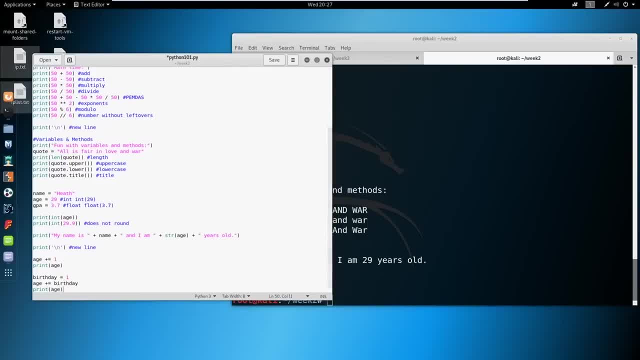 And if you printed age here, I would now be 31.. We are going to be going over functions. We're going to hit functions pretty hard and functions are coming up next. So actually that is it for this little section. We're actually going to hit functions right now. 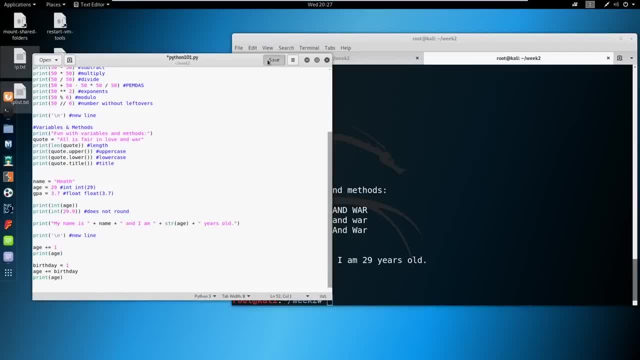 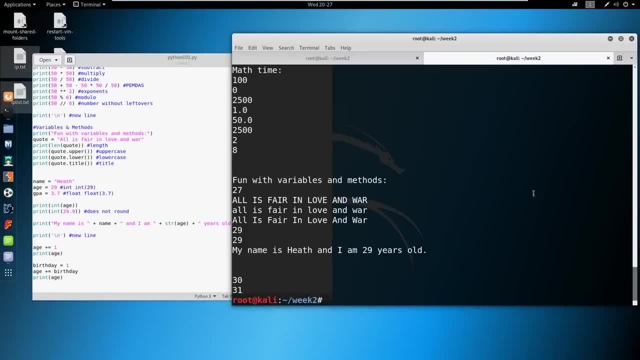 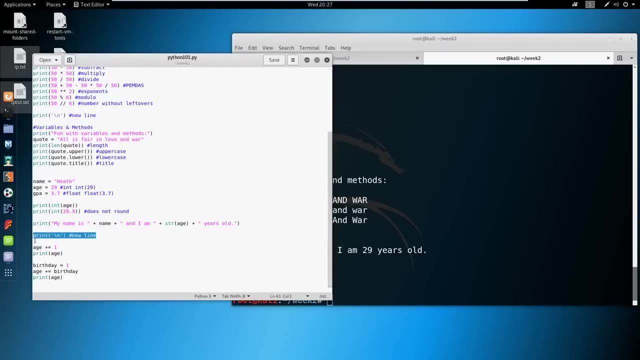 So good timing on that question, So we can save this. Just prove out that we've hit 30 and 31,, which we did. Okay, And now what we're going to do is we're going to dive into functions, So let's go ahead and just print out a new line again. 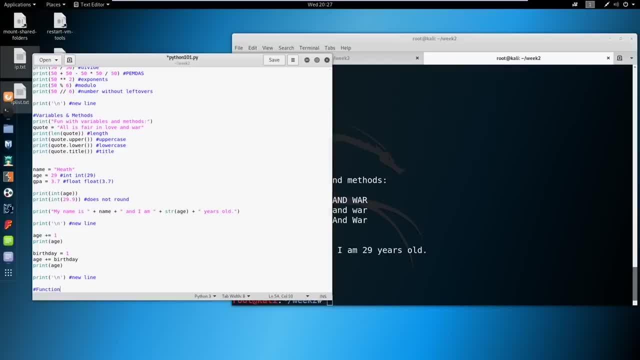 We'll call this functions. We are doing an AMA after this. Yes, There will always be an AMA. I need a drink, So give me one second. guys Talking too much, Okay. So now with the function. when we talk about functions, we talk about doing something for. 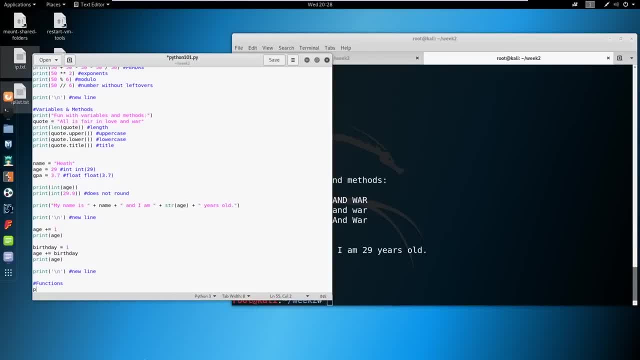 us. We're talking about a whole line of code in one defined area that we can call back at a later time. So if we're doing something repeatedly in our code, it would be better to actually just write a function for that and so that we can just write that code one time and call the. 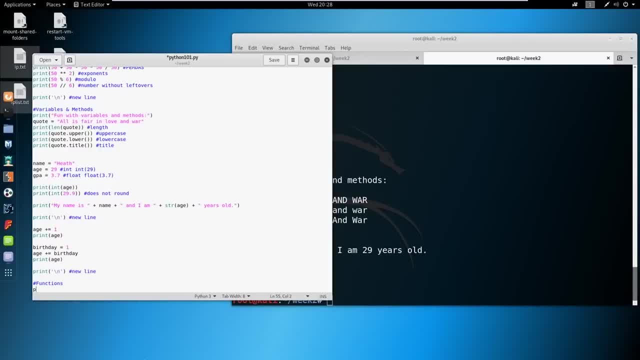 function later or repeatedly that we need to then to write out this code block and have a long code for no reason. So that's kind of the point of functions And it's going to make a little bit more sense here in a second. So let's print out: 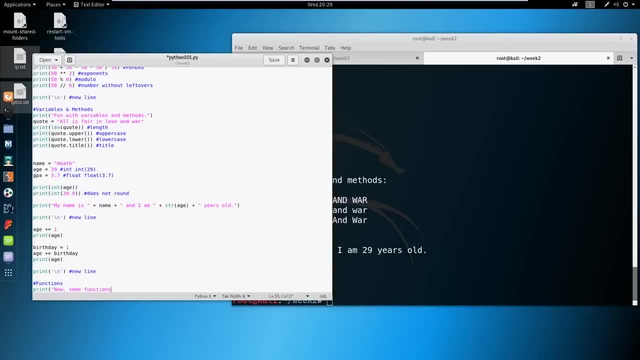 We'll just say: now some functions. Okay, So we're going to say define, We're going to call this Who am I? And now this is where everything comes into play, where it comes into spacing syntax tabs. This is something that's very, very particular to Python. 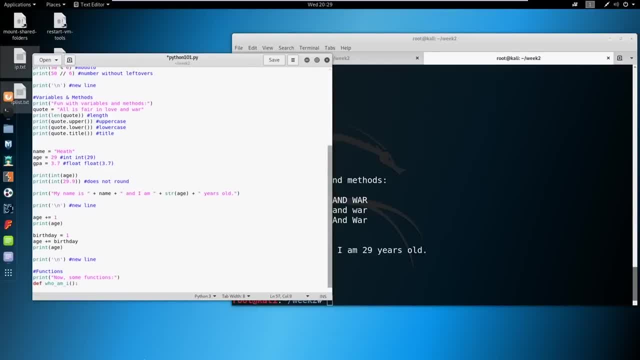 So we're going to hit enter and we're going to hit tab. Make sure to hit tab, or else your program won't work correctly. Make sure you also have the colon as well. So we're going to say: name equals Heath similar to before. 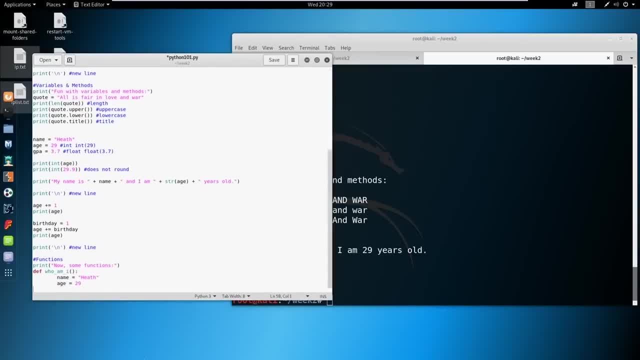 Age equals 29.. And then we're going to print the same thing from earlier. I'm just going to copy and paste it all into one, Okay, So now we can call the function with just saying who am I? Okay, And then we're going to print it out like that, right. 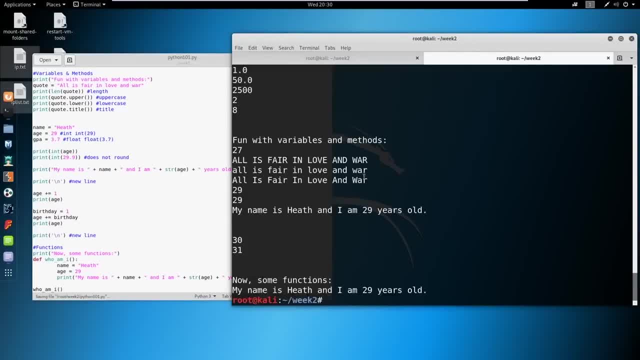 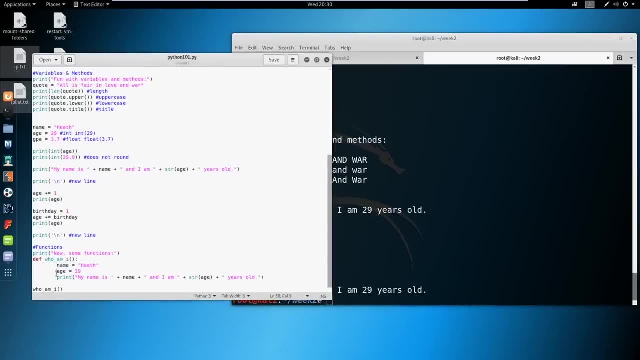 So if we save this and print it out, let's see if anything happens. Okay, It returned the function. So what happened is we declared a variable, we declared another variable and then we printed something out. Then, when we called this function, everything inside of it happened. 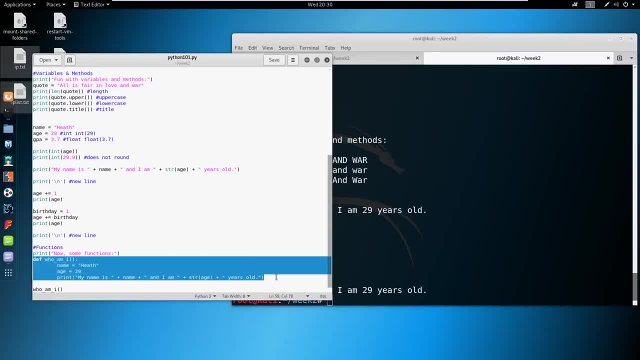 So what this means is everything that lives inside this function, stays inside of this function, and that'll become more apparent as we go. If I were to call, if I were to set the name, okay, let's just say, let's call this name. 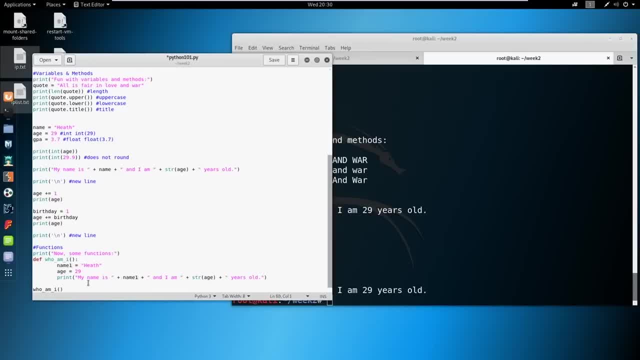 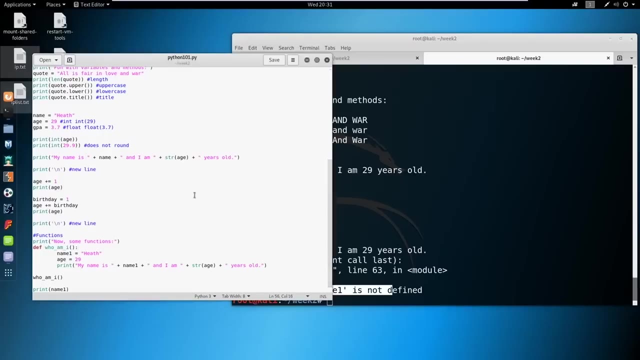 one, and we'll make this same here. We don't have a name one variable anywhere, right? So let's just say print name one, We say save and then we try to print. There's not a name one defined, because name one actually resides in the function itself. 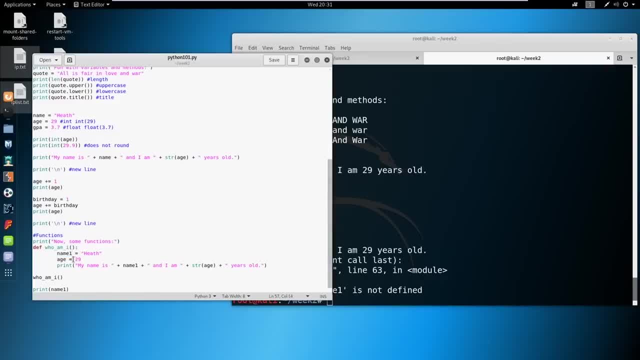 So make sure that you know that If you're declaring a variable for the first time here and it resides in your function, it's only in your function And thanks for those of you who are helping with the code that understand it. I don't have time, with as much as we've got to cover, to answer everybody's questions. 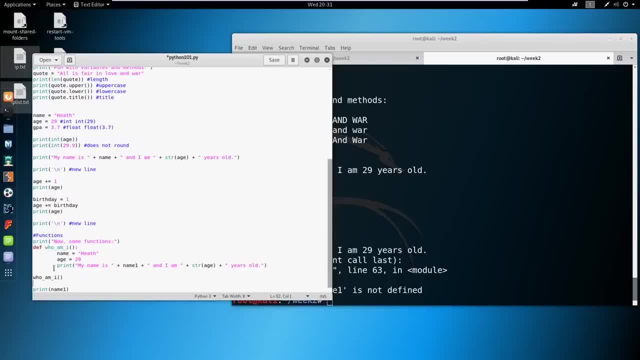 so I really appreciate you guys helping out with those questions. Okay, So let's go ahead and delete this print name one. We don't need that. So we can actually also call parameters, right? So let's take a look at what a parameter might look like. 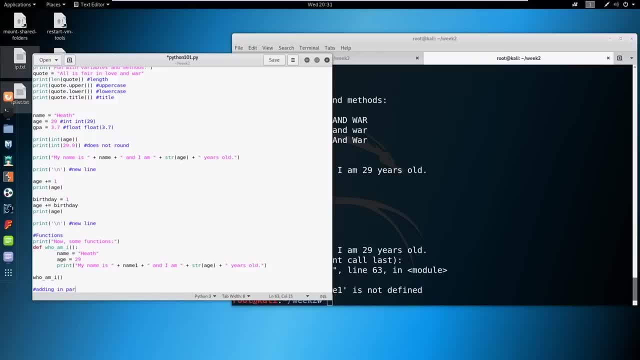 And we'll just put a little tag up here that says adding in parameters. Okay, And we're going to define a new function And this is going to be really simple. This function is going to be called add 100. And we're going to say the parameter is called num. 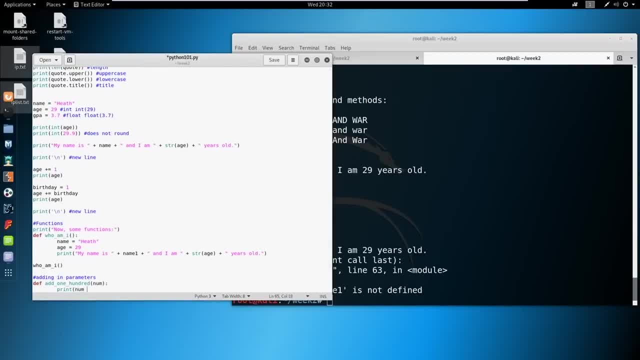 And what we're going to do is we're going to print a number, that parameter num plus 100. And that's it, So our function. all we're doing is we're giving it a number and we're going to add 100 to it. 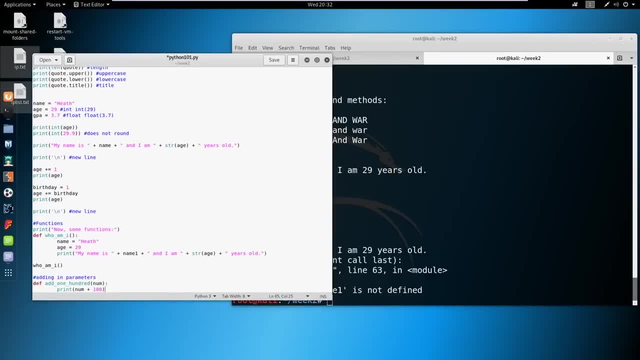 So it's a very, very simple little program here. Like somebody said, it's a mini program. That's really what it is, Okay. So now, if we call in add 100 and we call 100, it's going to be 200, right? 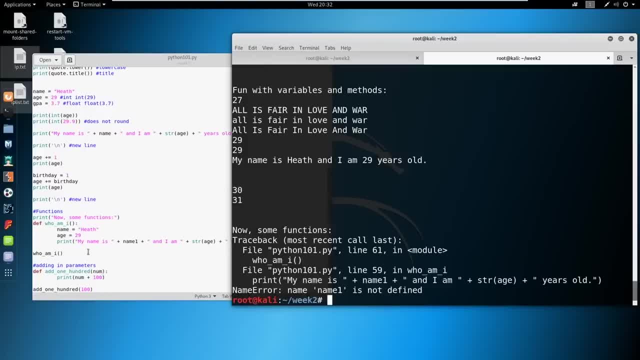 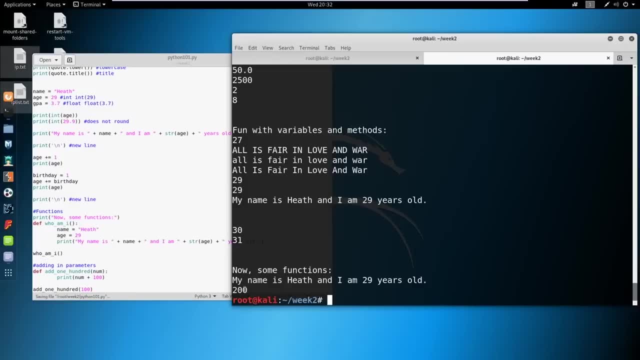 Let's print it and find out. We still have name one somewhere. Where did I put it In the string? I took it out of there. Try it again. See, now we're at 200.. Okay, So just think about these as little mini programs. 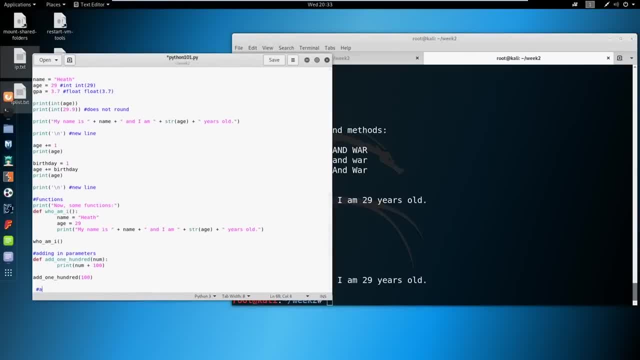 We can also add in, though we can add in multiple parameters. So what if we define something like add x and y, And then we just wanted to print out x plus y. Okay, So that's our little addition program, right? 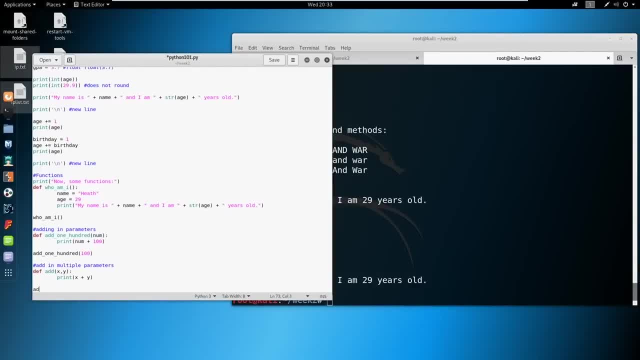 Not to say that Python doesn't already do it, but this is just for proof of concept. Let's add 7 plus 7.. And let's add 305 plus 207.. I don't know, And not with the plus sign. 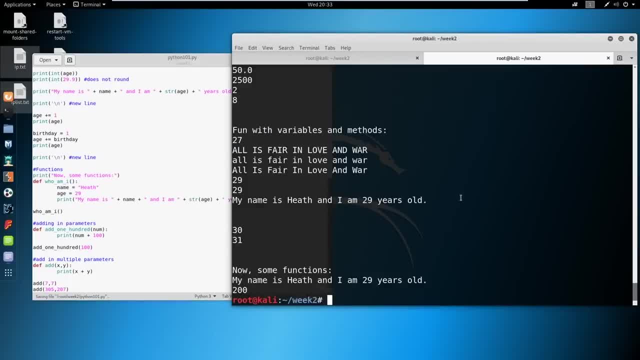 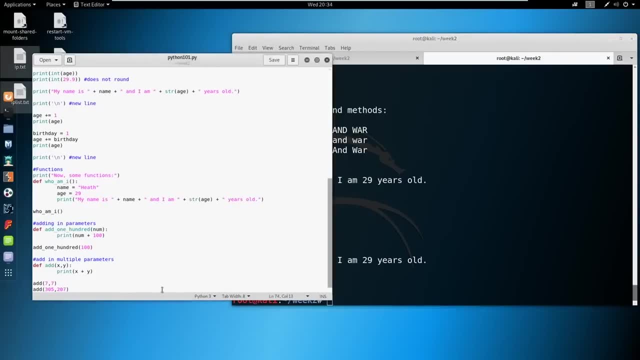 With a comma. Okay, So we've got that. We got 14,, which is correct, And we got 512,, which is correct, So we can also use something. This whole time now, we've been using something called print, right. 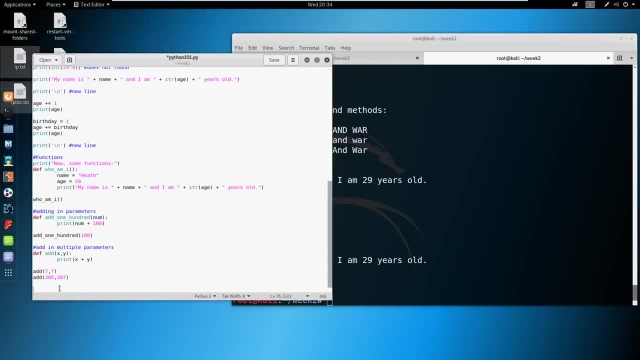 But we can also do something called return, where we return the value and we store it for later. So let's talk about using that. We'll say using return, Okay. So let's say define, multiply. We'll call it x and y again. 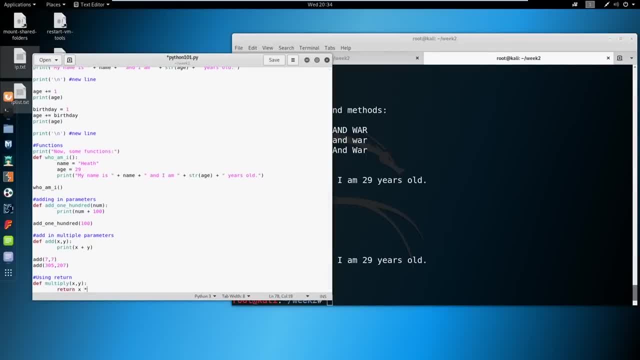 And this time we're just going to return x times y. If there's another heath in here, that's awesome. You're probably a good looking dude Just saying Okay. So now, if we wanted to print out that information, we could say print. 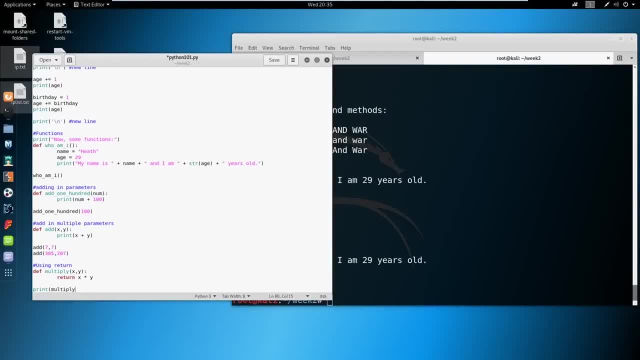 Okay. So let's say print multiply, And then we can give it 7,, 7 again if we want. Let's see if it's 49.. Just take a look, Okay, And we got 49.. We could also make a program called square root. 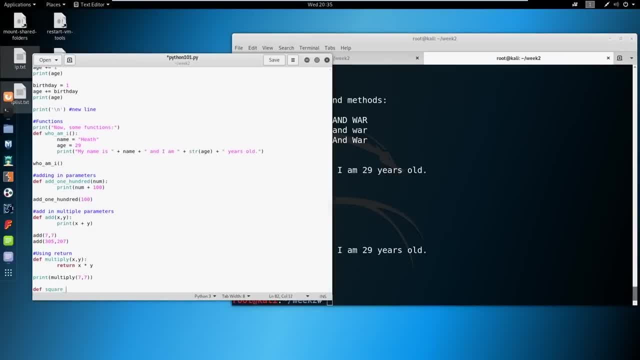 Let's try that. So if we say: define square root, Well, let's give it one parameter of x. What if we return x to the exponent of 0.5? Okay, So now we say: print square root of 64.. 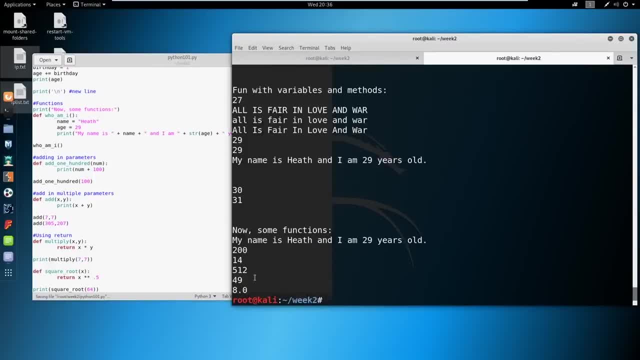 Save this And we get 8.. We actually get a float of 8.. And that's it on the function side. How are you feeling about the functions? Who was it asking? Was it Dodo While I take a drink and stall for a second? 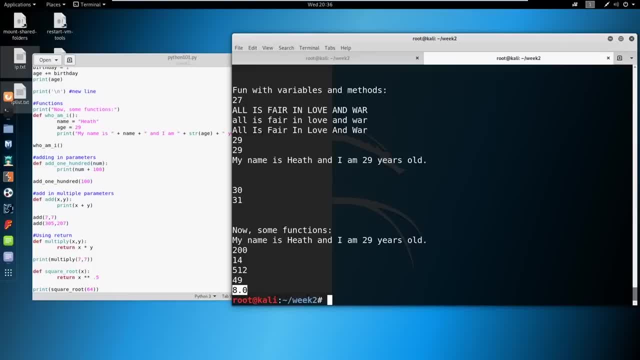 Okay, Let's see. Yeah, if we do IDEs, we'll get into those next week, if we do another week. But IDEs are very nice. IDEs nuts Nice. I like it All right. No complaints on the functions. 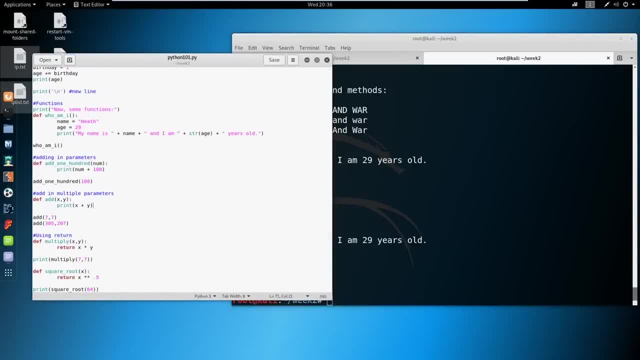 We're going to go ahead and move on. So we're going to be talking about Boolean expressions next. Let's go ahead and add a new line here, Call it Boolean expressions, And then we'll also imprint this. I'll just put true or false. 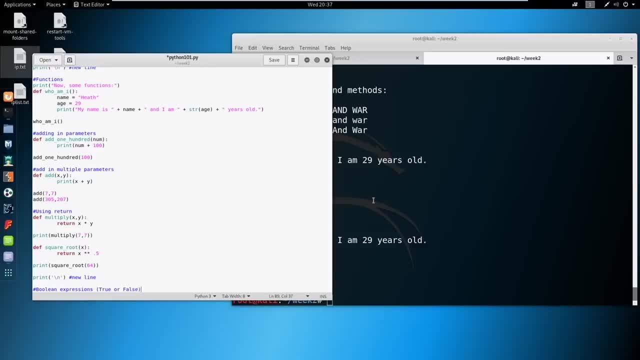 And note that true and false are capitalized. I should have a function for a new line. You're so smart, See. this is why White Rose gets paid the big bucks. I'll let you guys do that. You can write a function for your new line. 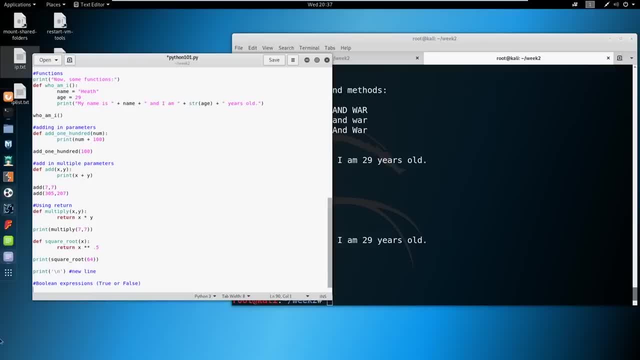 Okay, so true or false. Note again that true or false is capitalized. So we're going to have a little print statement. because I like the little title here, We'll just call it very simply: boolean expressions. Okay, we're going to print out a bunch of bools here. 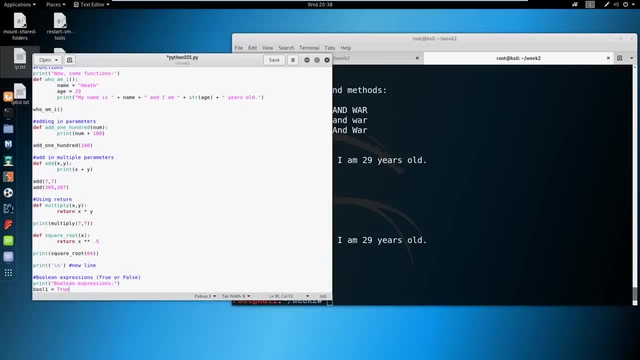 So we'll call bool1, we're just going to call it true. but what about bool2?? We'll make bool2,. what about 3 times? like a type, 3 times 3 is equal to 9? That's also true. 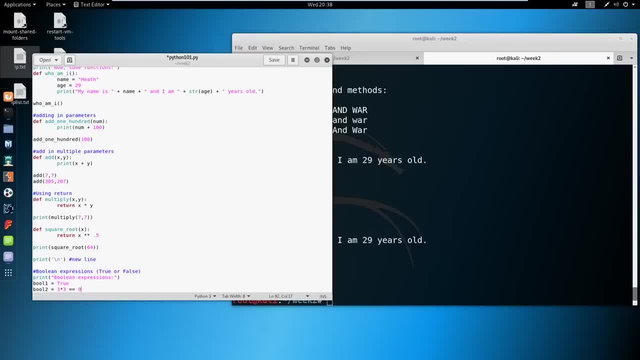 And notice what I did there. The two equals is an equal right. If you have the one equal, we're talking about a variable. So make sure, if you're doing an expression, That you're setting it with equal, equal. Okay, let's look at a couple more. 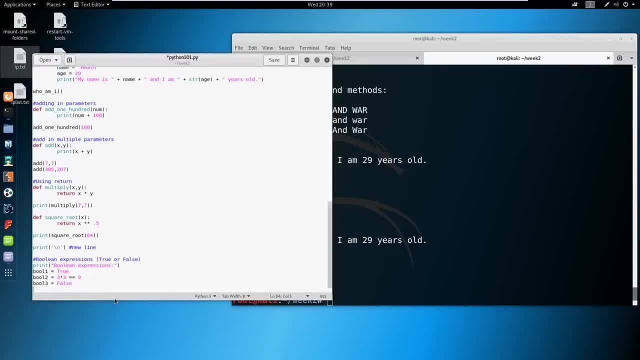 bool3, let's just set that to false. And bool4, let's call this: 3 times 3 does not equal 9.. So that's also false, right, And? And we can do a quick check. we could say: print: bool1,, bool2,, bool3,, bool4, okay. 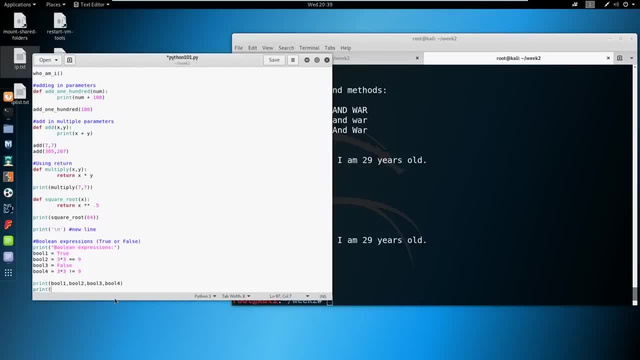 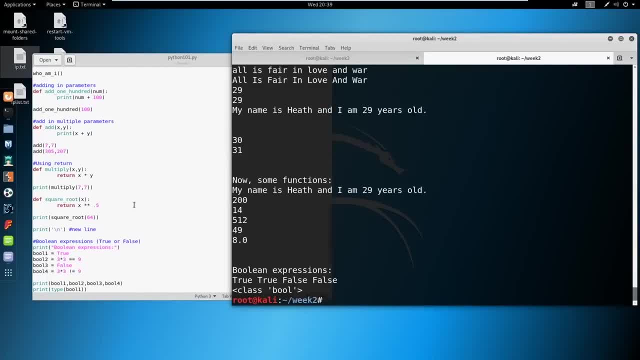 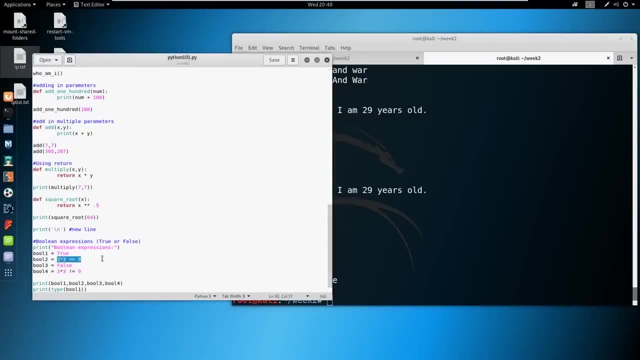 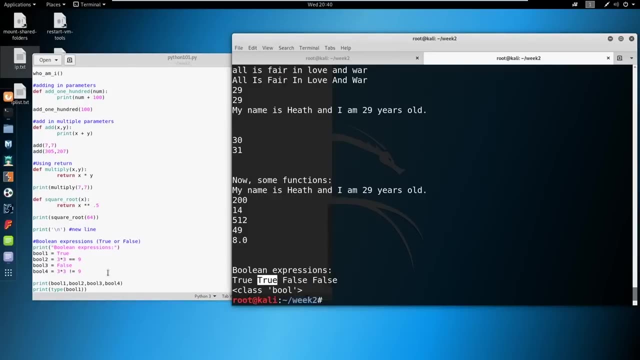 Okay, So, as expected, true, true, false, false. So you see, even though we put in this equation here, It's not doing any math, It's checking for whether it's true or false, So it did come in as true. 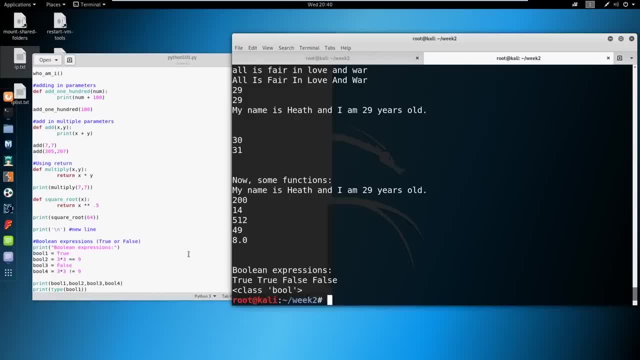 And this expression came in as false In. the thing I wanted to show you here was: when we have this type, This type becomes important. right, You can check what kind of type the class is. This class is a bool. But what if? 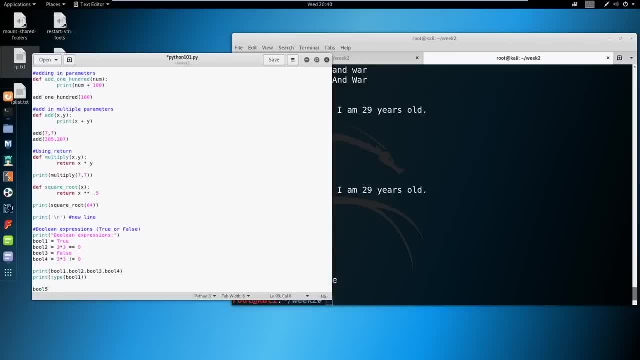 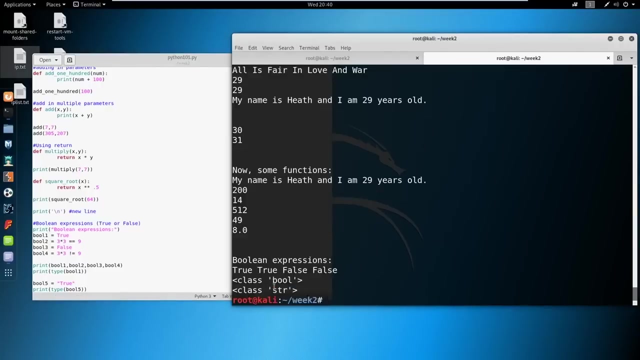 put bool 5. and we said it was equal to true. like this: What does that become? I'm sure everybody gets this right. Or bool 5. Becomes a string. that is correct. Class changes: It's a string. 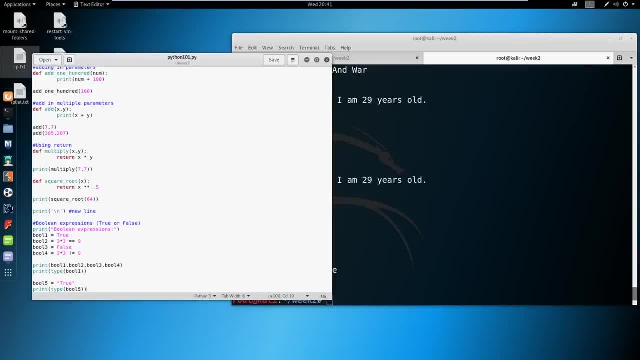 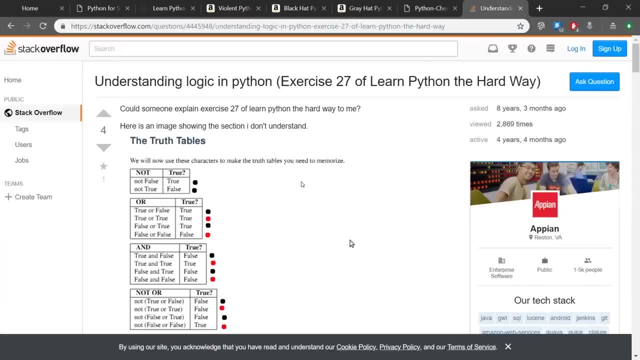 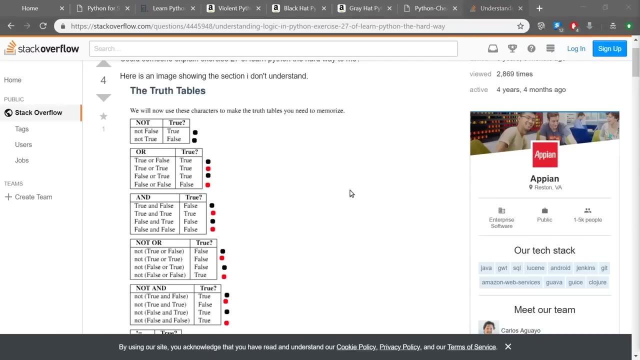 Okay, So there are these charts. Let me pull one up for you. I think they're called truth charts, Truth tables, Where we'll get into this in a minute, when we get into our statements. right, We're going to talk about operators in just a second. 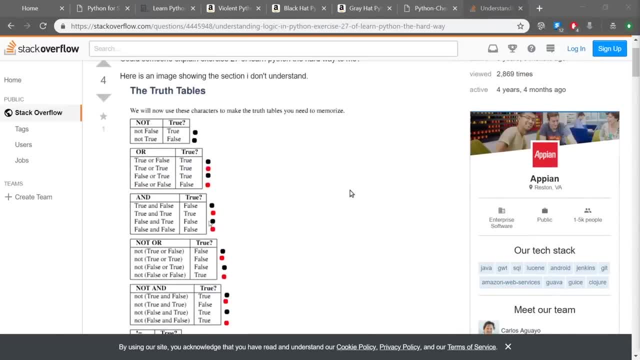 And then we're going to talk about these charts, But we're going to get into these, not or and. And then we have these true or false, true and false. And it'll get interesting in just one second, So let's dive into that. 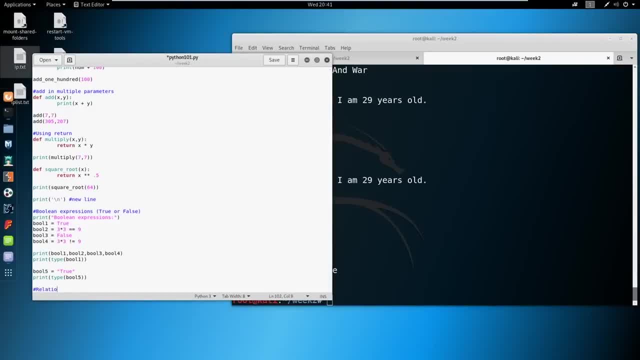 So what we're going to call these are relational and boolean operators. Okay, So let's create some variables real quick. Let's say: greater than is equal to 7, greater than 5. And less than less than is equal to 5.. 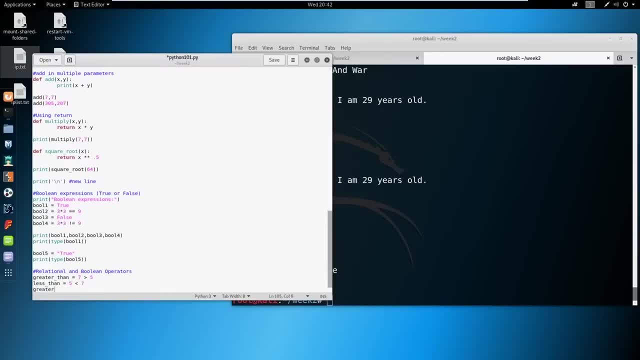 less than 7.. This one's going to be a long one. Greater than equal to is 7.. Is greater than or equal to 7.. Or less than or equal to 7, less than or equal to 7.. 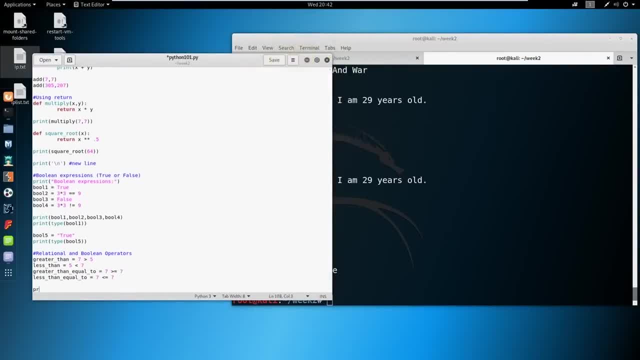 Now, hey, thanks for the sub, Jake Appreciate it. So if we print all this, which is a pain to type, I could have made these shorter. I tried to make it logical. We hit save, Print it. Everything is true. 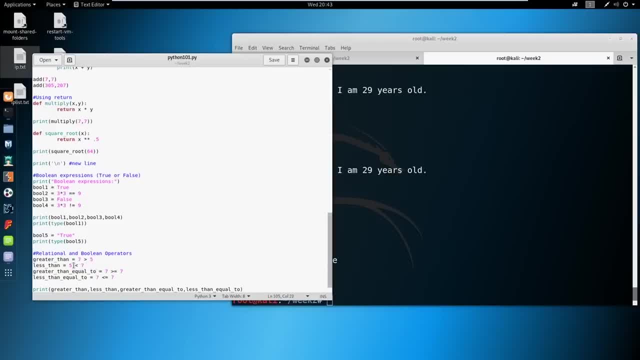 So I threw some new operators at you here. Right, We've got greater than, less than, greater than or equal to, less than or equal to. Let's throw a couple more in there. Okay, let's call this one test, and. 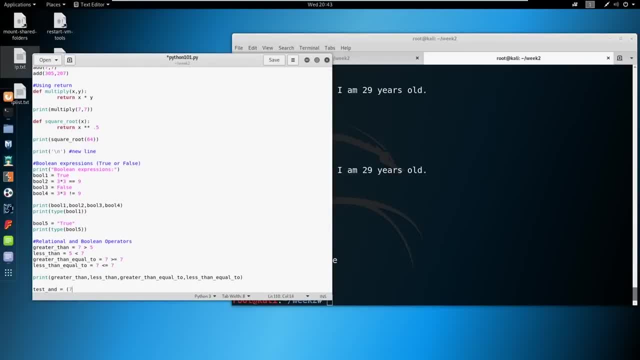 we'll make it shorter And we'll say 7 is greater than 5. And 5 is less than 7.. We'll cover these in a second. I'm just going to type it out: Test or: 7 is greater than 5.. 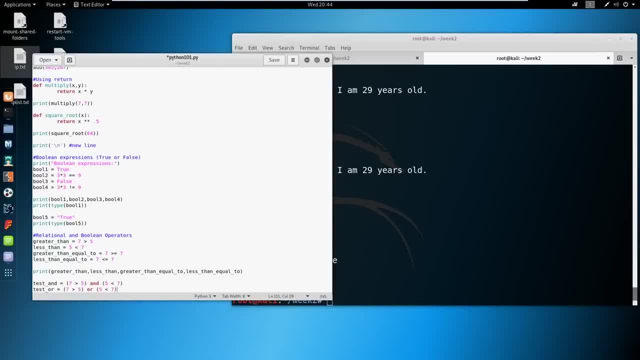 Or 5 is less than 7.. Test not. We'll just say not true. Okay, So we have these statements here. We said 7 is greater than 5.. Okay, that's true And 5 is less than 5.. 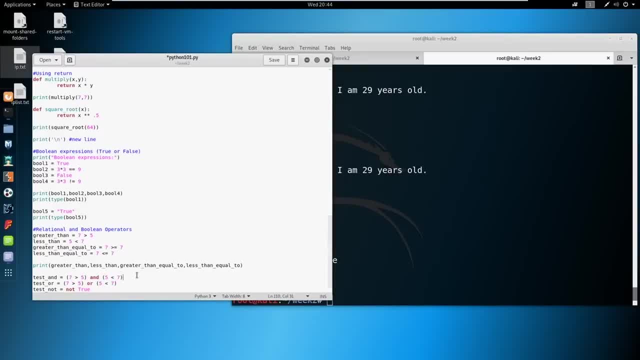 And 5 is less than 5.. 5 is less than 5.. 5 is less than 7.. Okay, that's true. So this would be a true statement. This would return true Now if we said 8 was less than 7,. 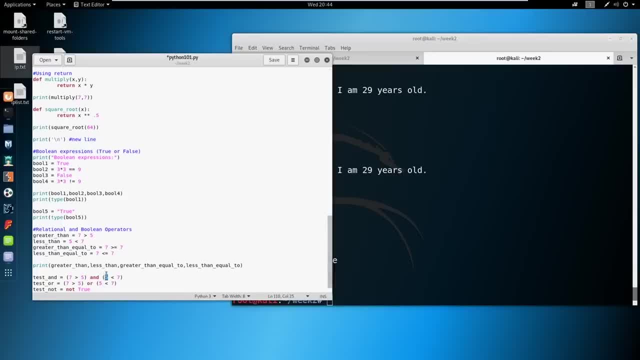 this would become a false statement. And that's where the truth tables come into play, right? Because for an and statement, both conditions have to be true For it to be true. if it's true and false, or false and false, then the statement becomes false. 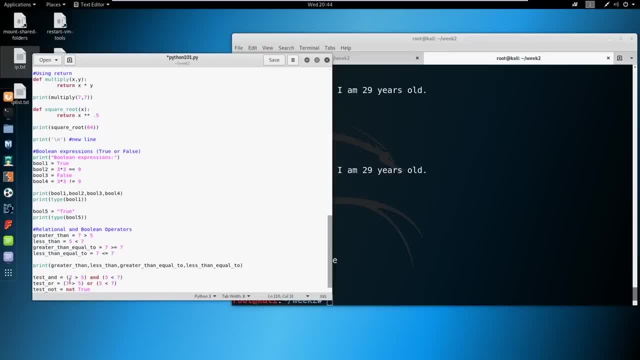 One false in this statement makes it all false. Now, if it's true or false, then we have: okay, true, we have true or true here, which is true. If we have true or false, it still remains true If we have false or false. 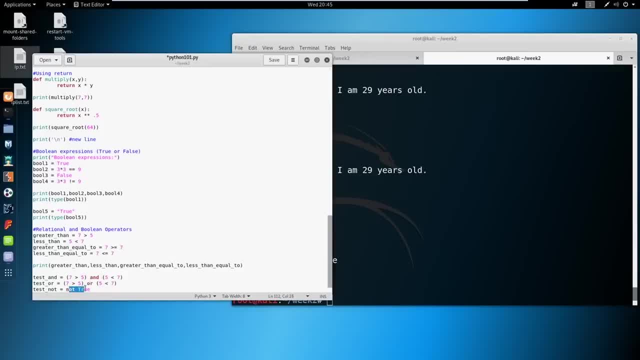 then it becomes false And then we have a not here. We say not true. Okay then that's false Or not false would be true, And we could check the truth tables and kind of go over those as well. Not false is true. 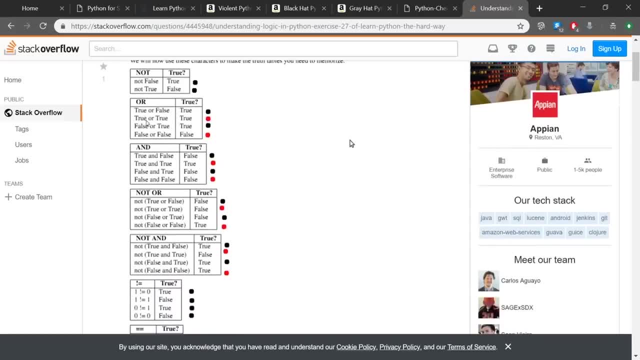 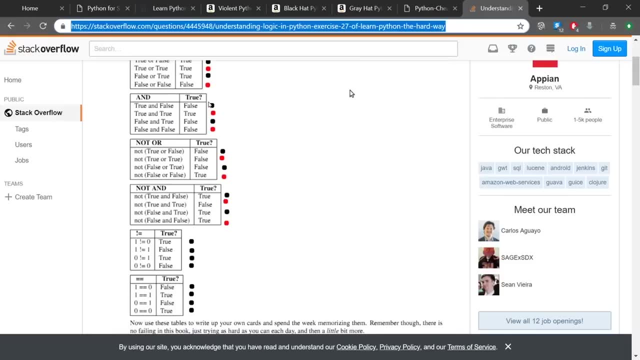 Not true is false. You see that True or false is true. True or true is true. False or true is true. False or false is false. And I'll send this out in the chat so you guys can see this. You are correct, White Rose. 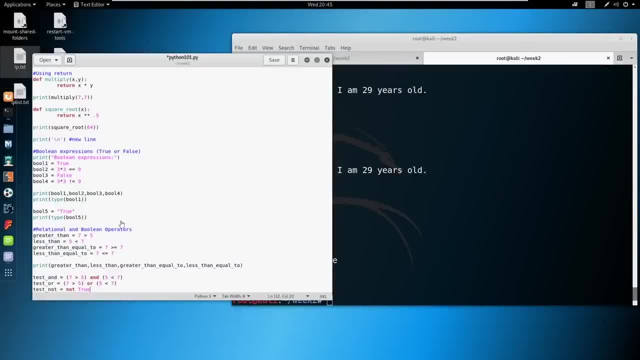 I should have had that And as I was typing that out, I was surprised that one of those was not, So that was my mistake. But White Rose is correct: One of these should prove that this would return false. So if we make it, 8 is less than 7,. 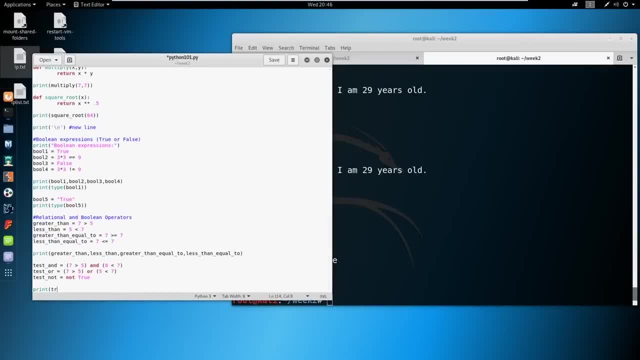 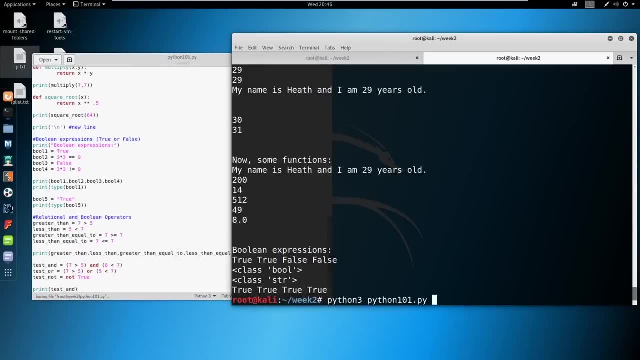 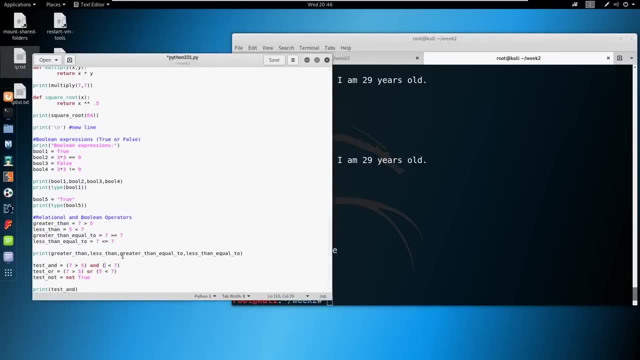 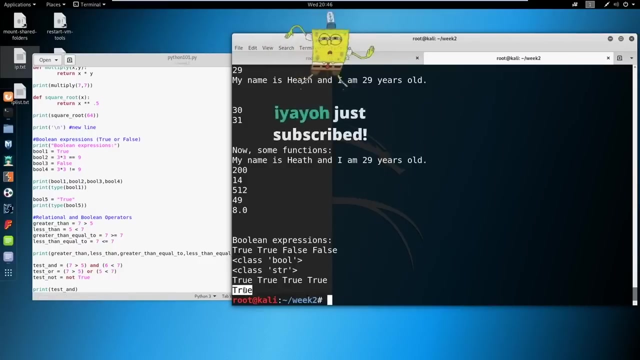 we can prove that Like this: If I could type- apparently I can't type And you see, it returns false. So if we made it 6, where both conditions are true, then it becomes true. Hey, thanks for the sub IAO. 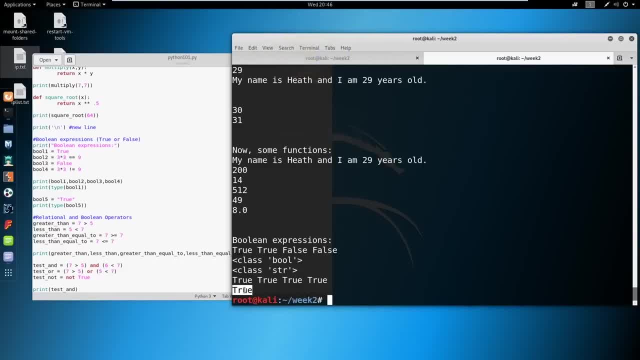 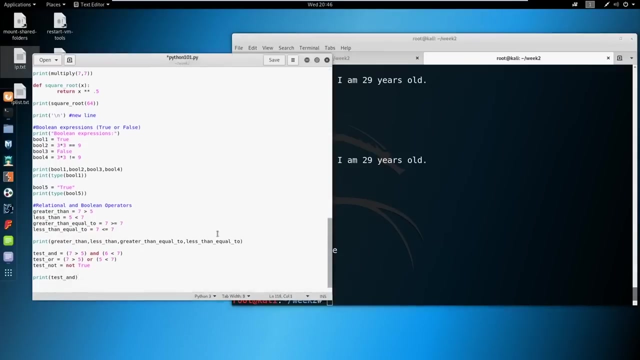 Appreciate that I'm starting to lose my voice. We're not even an hour in, guys. I'm weak. Okay, I'm trying to keep my sultry voice. I'm trying to. All right, I'm still going to copy and paste. 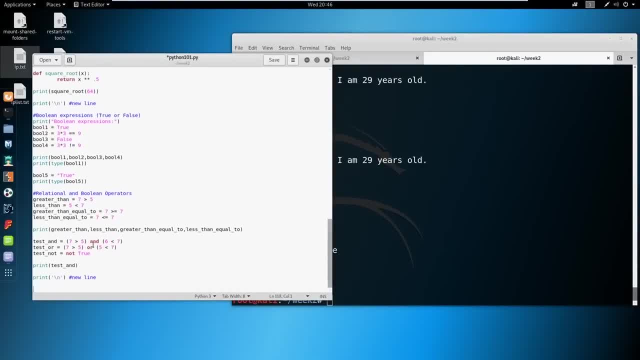 You guys aren't going to change my ways. All right, Let's talk about conditional statements. I'm just going to print out conditional statements. I'm going to write to you guys and see what happens. Okay, Let's see. Let's see. 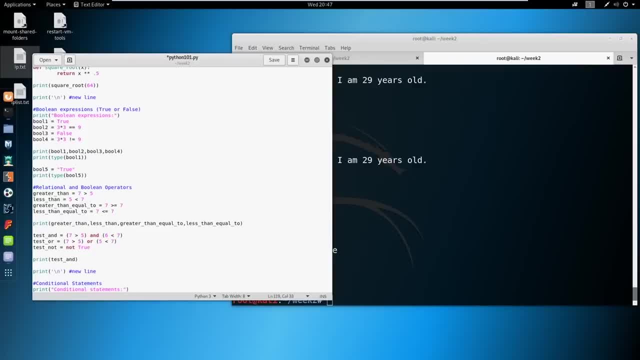 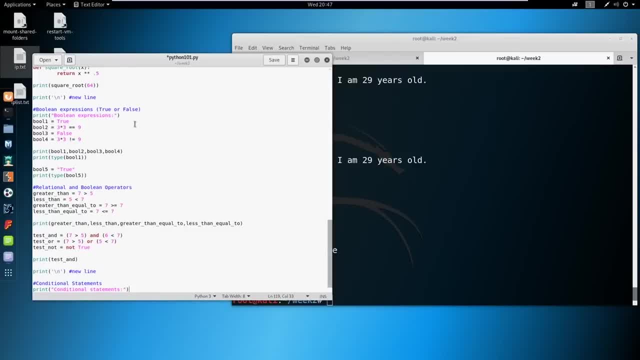 Is everybody able to see this on like a full screen level, Or should I try to boost this up? I don't know what the options are for that A tidbit. I can zoom in a tidbit If I know how to zoom in a tidbit. 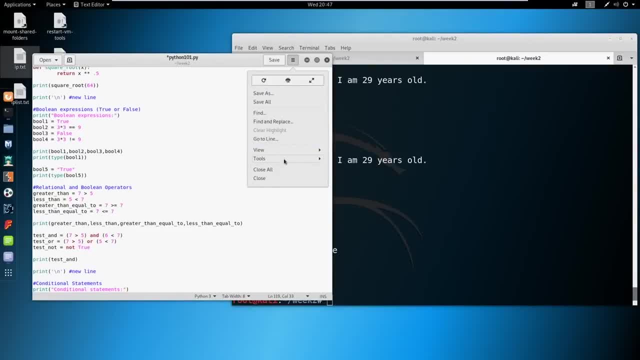 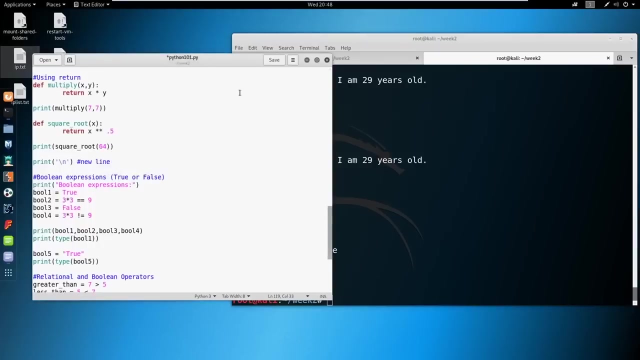 Somebody knows the way. Text editor and top bar. Oh, you guys are awesome, All right, Aha, You guys are the real mentors. Look at you. Actually, I'm still going to keep this lowered. Is that better? Better one. 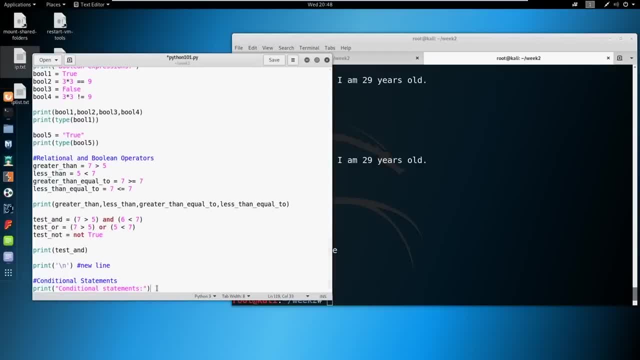 Better two. Okay, Sorry, guys Will note for future lessons a tidbit better, Okay. All right, let's do some conditional statements. We are going to do if or else, and we're going to try to buy a soda. 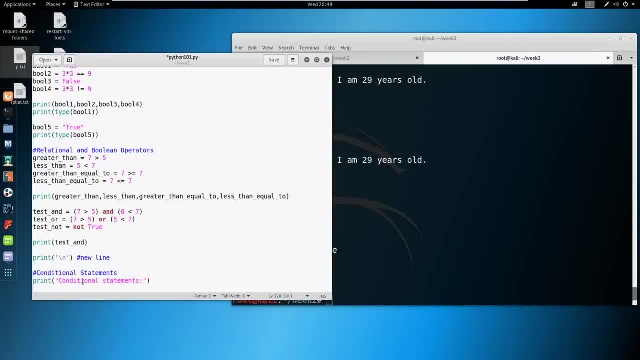 I don't like dark, I like light. All right, so let's define a function. We're going to call it soda and it's going to take one parameter called money, And I want to buy this soda, But I want to buy this soda if I have enough money to do it. 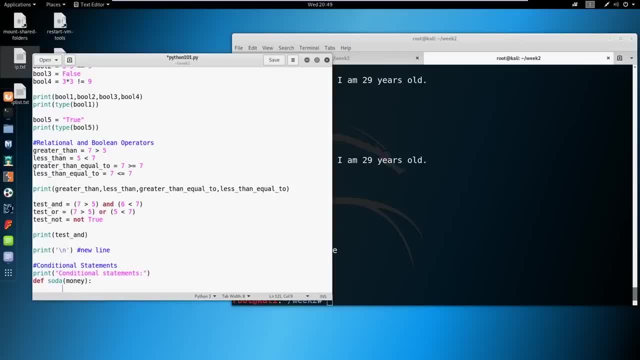 So let's say the soda costs $2.. So if I want to buy the soda and I have $2 or more, then we can return. you've got yourself a soda And I keep doing it, caps locking. if we don't have $2 or more, then we have an L statement. 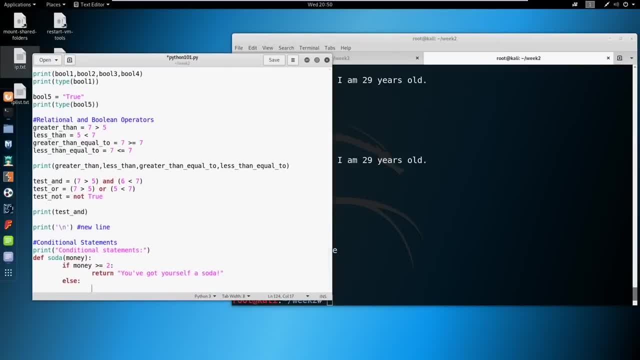 So if one thing is true, we're going to return one thing else, we're going to return something else. It's a pop if you're from like Ohio, Michigan, Maybe Kentucky. Yeah, Yeah, Yeah, I don't know. 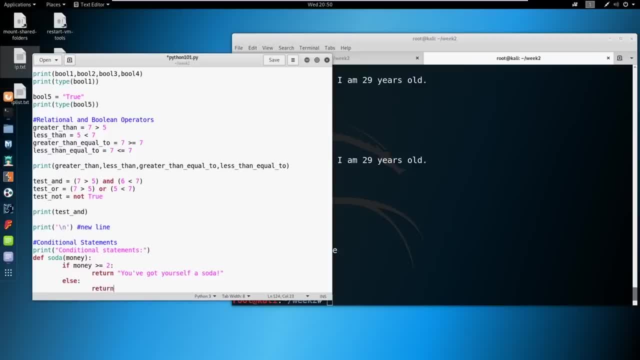 What are the chances? those people are here right now. Here, we're just going to return: no soda for you. Yeah, They don't have the internet. Okay, So let's print out soda and say we've got $3.. Let's also print out soda and say we've got $1.. 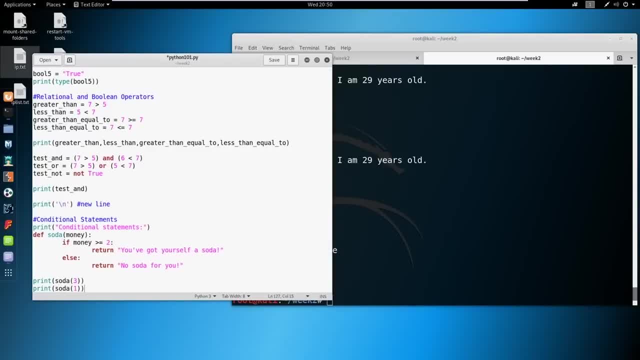 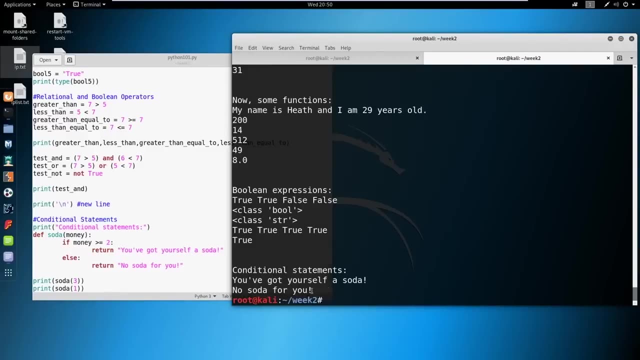 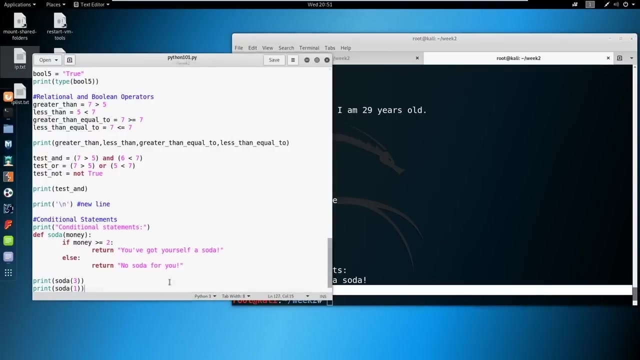 Cool. All right, That's a big one, Cool, Okay. you see, with $3, we've got ourselves a soda. If not, we do not have a soda. Okay, Let's do one a little bit more complicated. 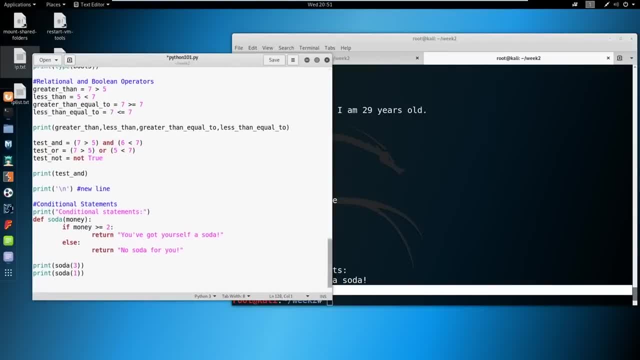 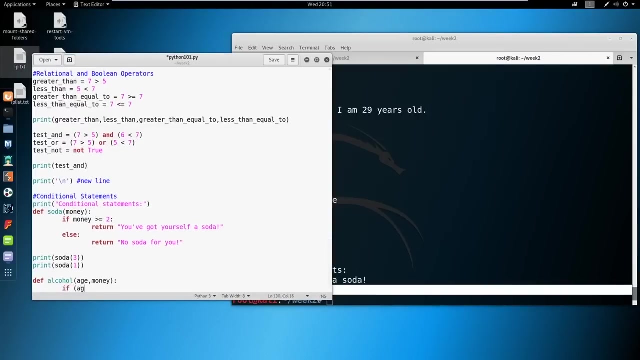 I guess not too complicated. So let's define one for alcohol. Well, we need money, but we also need to be of age, right? So if our age is greater than or equal to 21, this is in the states, The states. 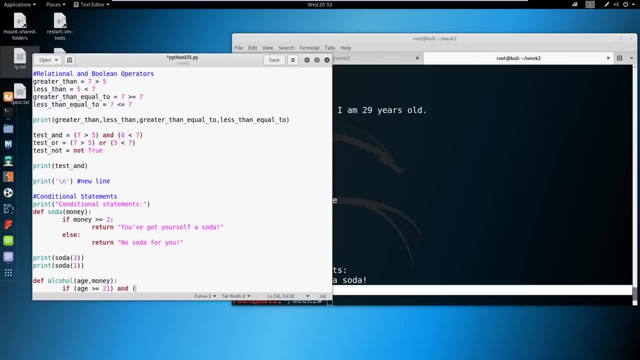 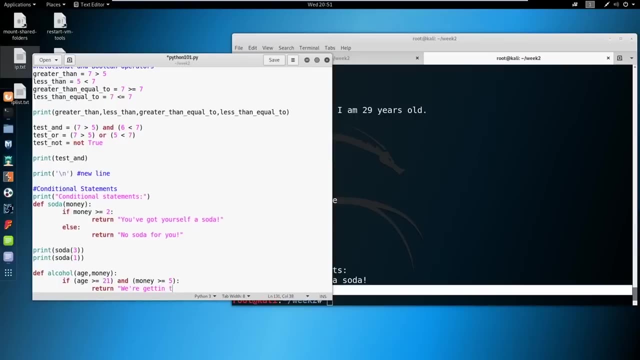 The states, people And let's say, the drink costs $5. Then we'll return. we're getting tipsy. If that's not true, we can do something called an else, if, If we have another statement. what are some things we need to think about? 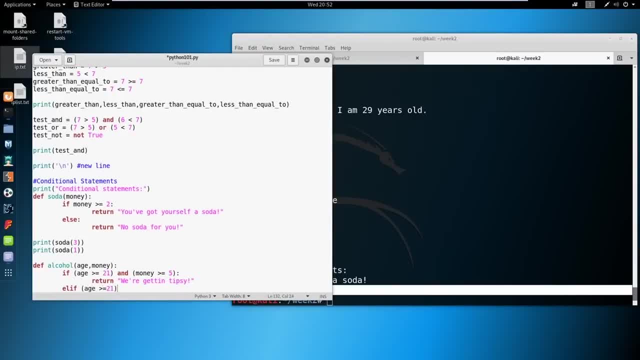 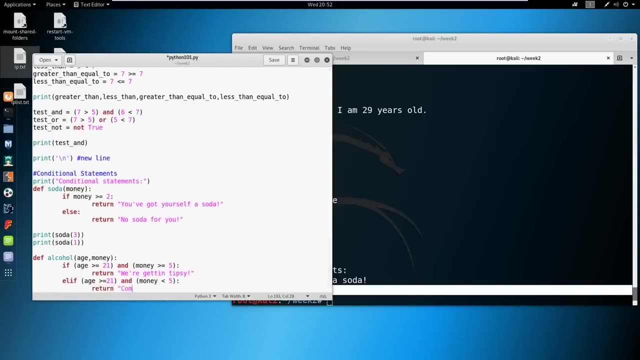 What if our age is greater than 21, but we're broke? Then we're going to say: return, come back with more money. Okay, What if we have the money but we're not 21? Well then we can return. nice try, kid. 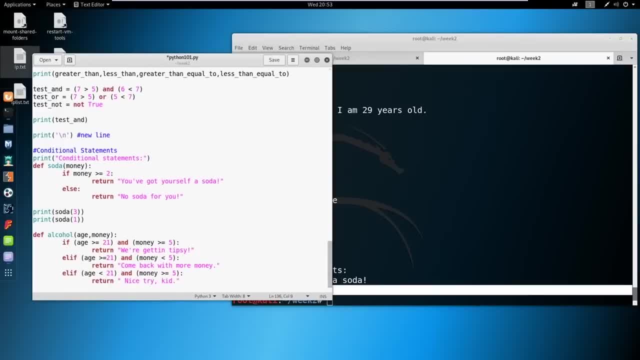 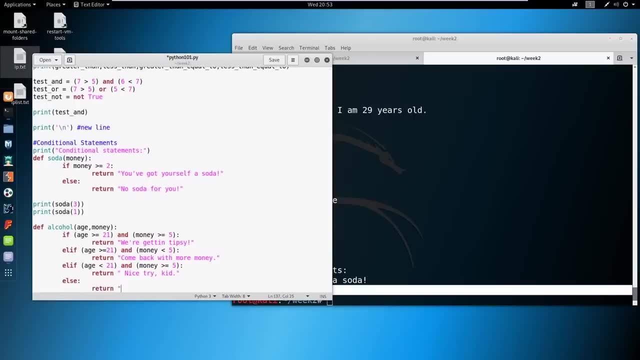 Right, Right. Lastly. Lastly, if we don't have the money and we're not of age, you're too poor and too young. I think you'd only want to print if you want to print to your screen. We're returning here because we're just returning the function. 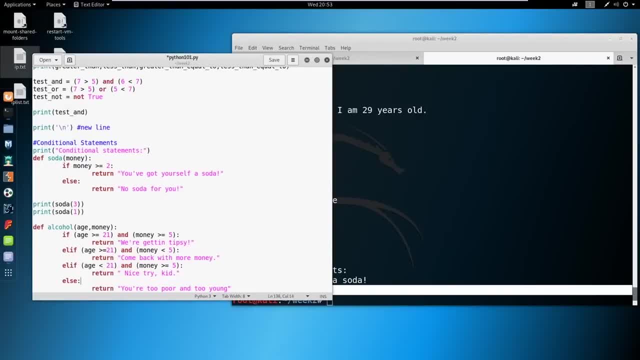 Okay, We're returning the- I guess the string, if that makes sense for what we're doing, but we don't have to print it out right now. But if you want to print out the results, then that's when you would use print if 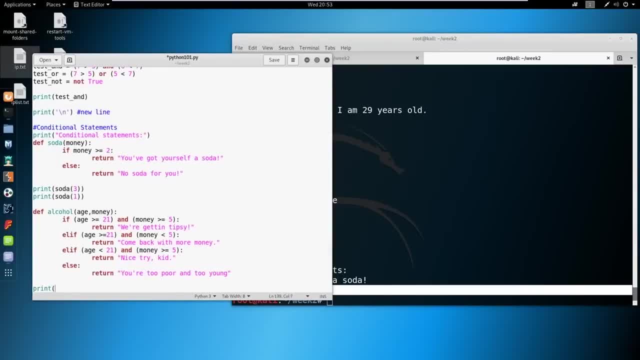 that makes sense, Okay, So let's print out some results here. Let's just test a few things. Let's say we're 21,. we got $5.. Let's also say we're 21,, we got $4.. And lastly, we are 20, with $4.. 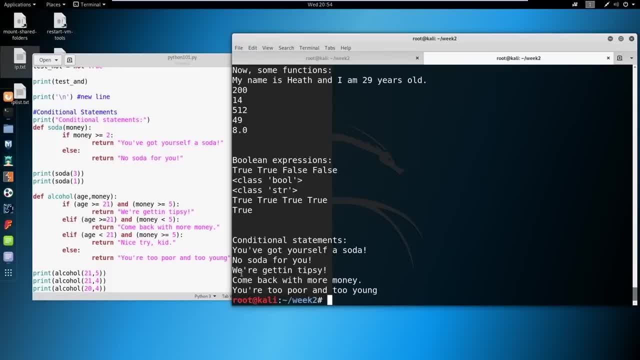 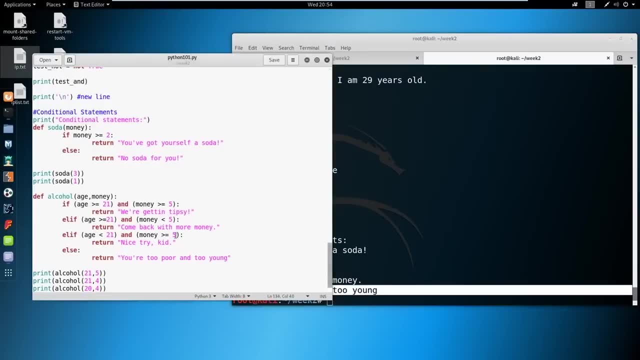 Okay, Save it and print So you could say it says: we're getting tipsy, Come back with more money and you're too poor and too young. Whenever people send you freely, popular showed up with a couple hundred dollars in short winnings. the number of people the customer saw was over 600 million. 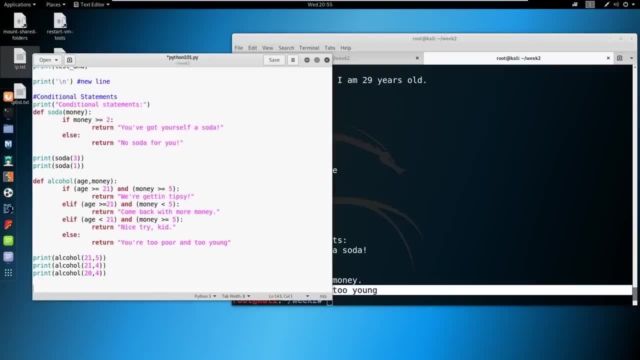 Animating the dollar from bleeding advertising. those were your yields. Thanks, Have a good time. All right, We're done. Thank you, Bye, Bye, Bye. Thank you, Bye, Bye, Bye, Bye, Bye, Bye. 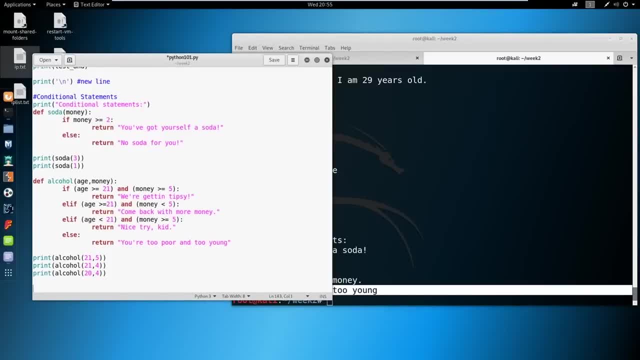 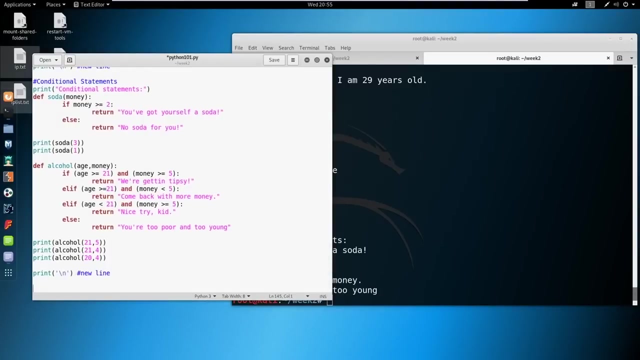 Bye, going through a little faster than I hope, which is good, though. We have a jam-packed night, No questions. Good, Okay, let me go copy and paste my new line, my copypasta, Okay. next we're going to be talking about lists. After lists, we're going to run into. 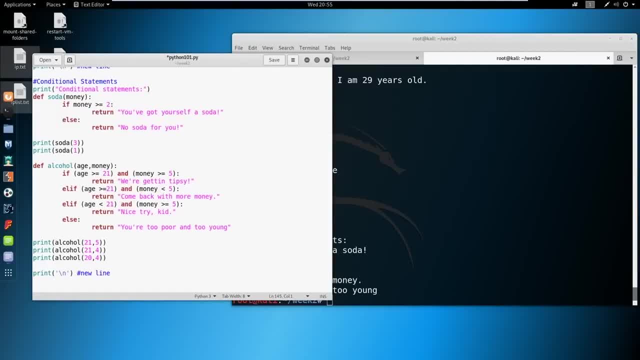 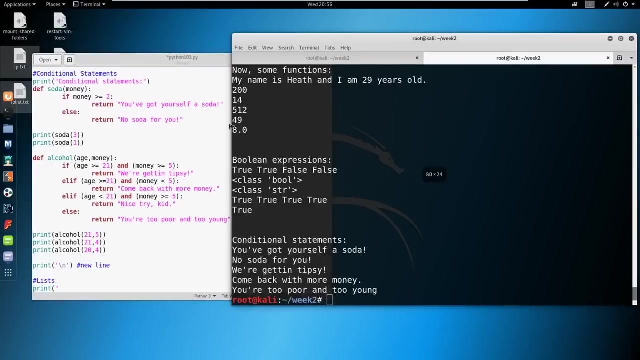 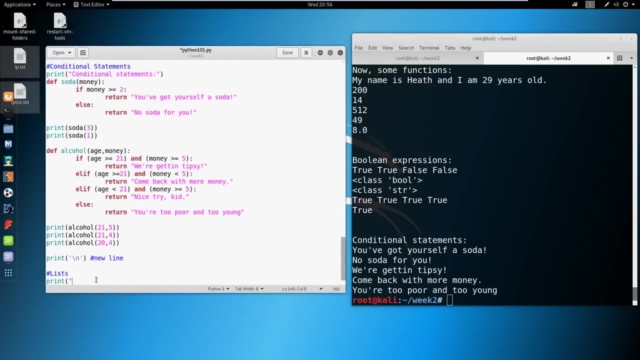 tuples really, really quick, and then we're going to talk about looping. So let's go ahead and say lists. Okay, print out a little friendly reminder. You need both. I can do that. There you go. Okay, so we're going to print out lists. 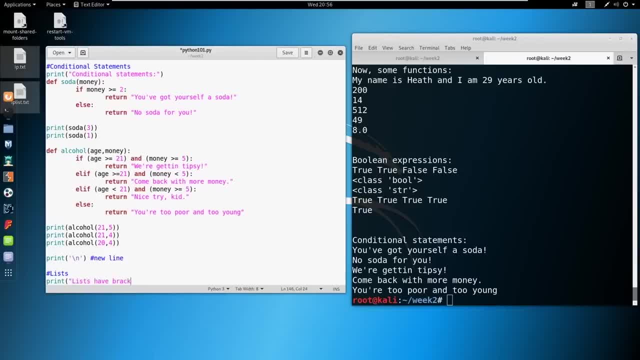 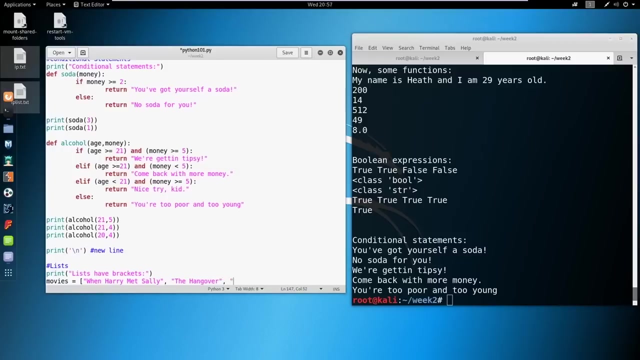 have a name, Have brackets. Let's make a list. I'm going to make a list of some of the movies that I like. Let's say When Harry Met Sally, The Hangover, The Perks of Being a Wallflower, The Notebook. 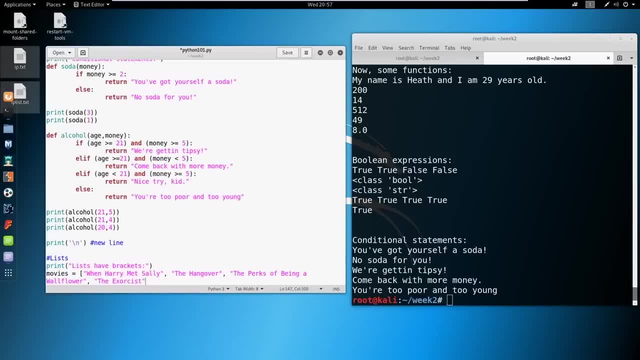 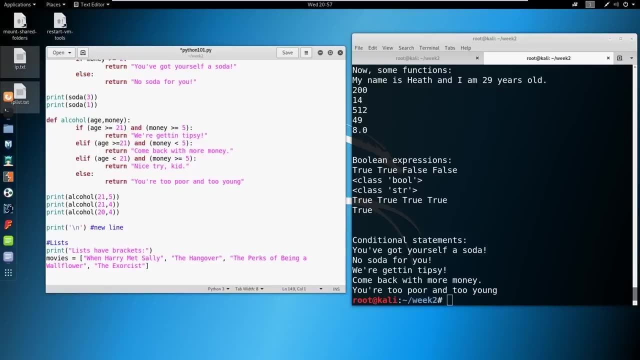 And The Exorcist, Throwing that one in there for Jeff if Jeff's in here somewhere. Okay, so we've got this list And we can do this. We can do lots of different things with this list. For example, let's say we wanted to return the first item in the list. 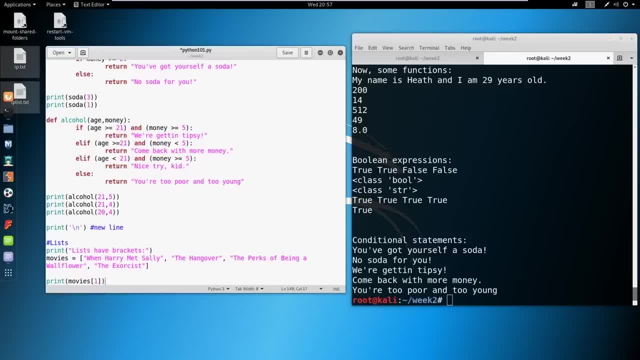 What do you think Would this do it? Let's print it out and see what happens here. We have printed The Hangover. That is the second movie in our list. Okay, So when we're dealing with a movie that's been posted on our list, 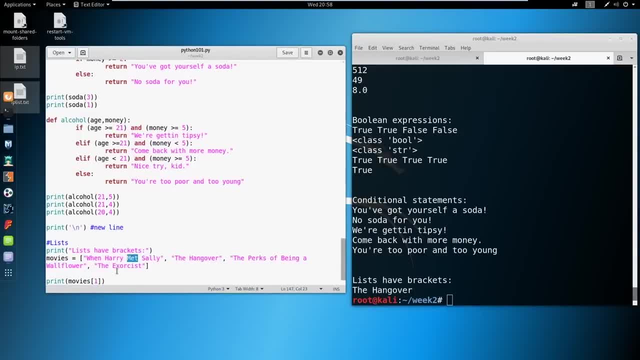 with lists and dictionaries and whatever else, we're going to be running from zero on. so one is actually number two, if that makes sense. so we want to print the first movie in the list. we actually have to call out a zero. hit, save on that and then you can see. 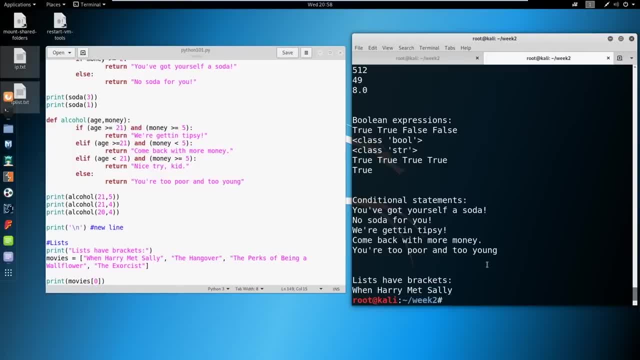 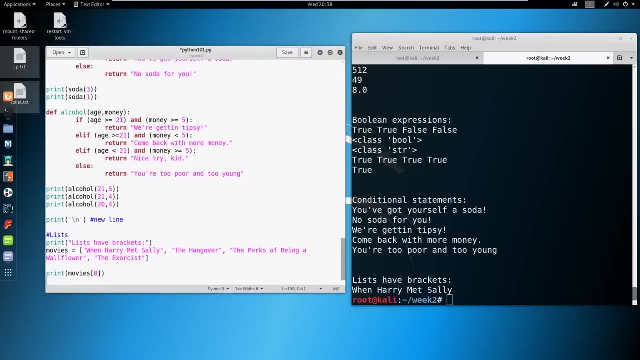 now, the first movie that prints is when harry met sally, so remember that numbering starts at zero. okay, let's say we wanted to pull a list here and we wanted to pull out of this list the first item and the second item. don't get ahead of me with negative one. we're getting there. 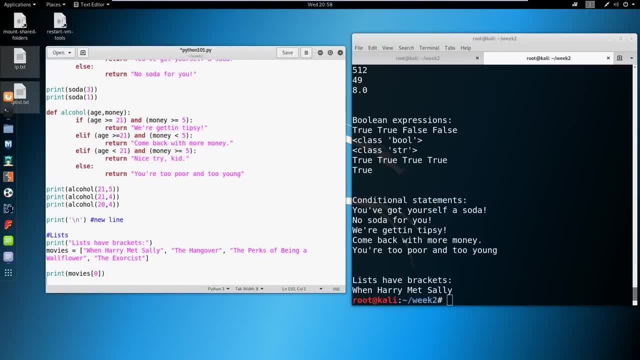 uh, so okay, let's say, if we want to get the first item in the, the second item, okay. so print movies do something like this: one to three. now this is weird too. right, okay, we did get the first item, or first. sorry, i said first item and second item, i meant second. 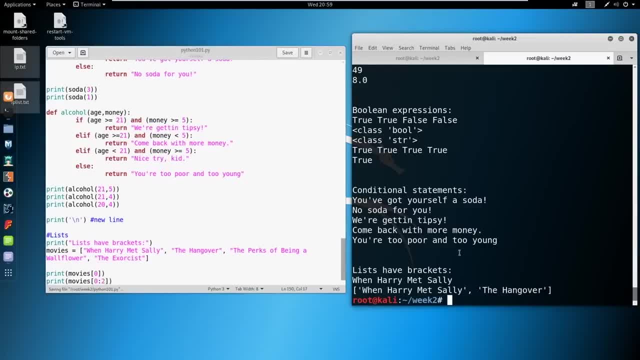 and third, but i'll switch it because that's the right thing to do. okay, so we pulled out when harry met sally and the hangover, but we called zero, one and two. well, this is a special case as well, right we? actually, when we want to call a list like this, we have to call out the next number as the ending. 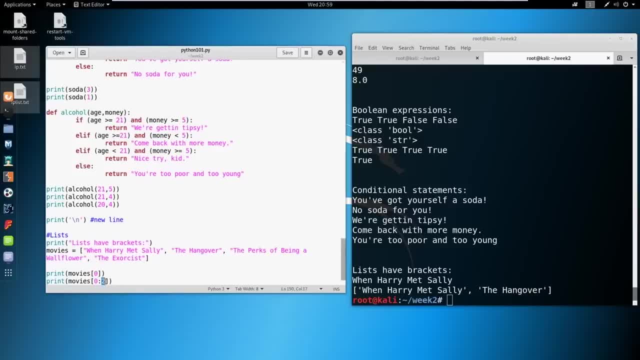 number. so we call the starting number we want and then one more than we actually want. so if we wanted the perks of being a wallflower in there as well, okay, we'll save zero. three print python 101, and now you see that we have three movies in there. 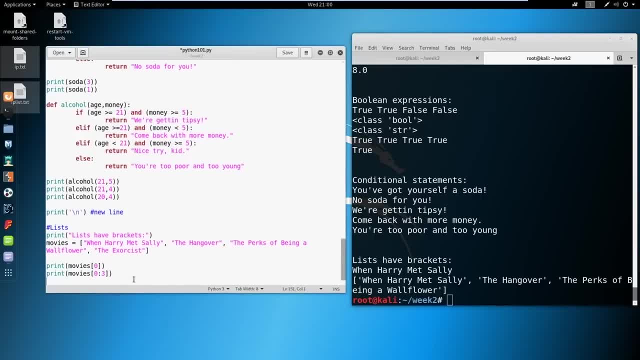 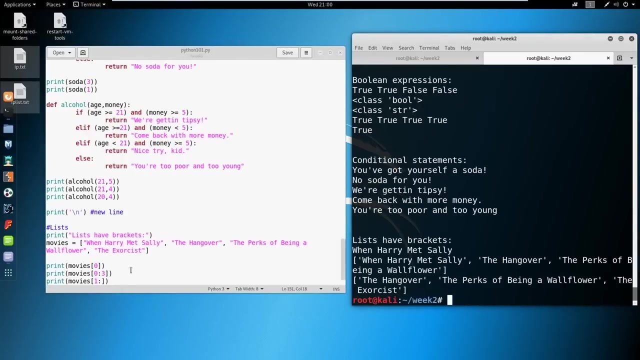 so it's a little funky. what if we did something like this- and this is called slicing, that's a great way to think about it up to, but not including thank you for that. what's this look like? so we're just printing out the entire list from starting point of one until it ends, right. 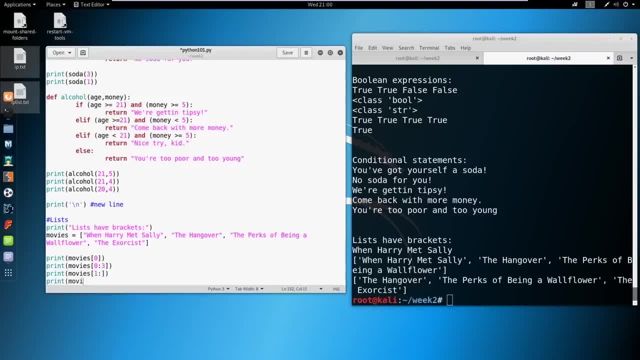 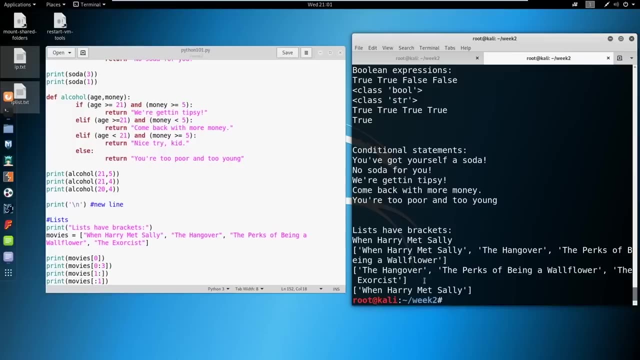 and what about if we print movies and we say something kind of opposite? okay, we just pull out when harry met sally, because we slice and we stop at one. so we're only pulling out the first movie there. okay, somebody already spoiled it. we won't name names, guys. 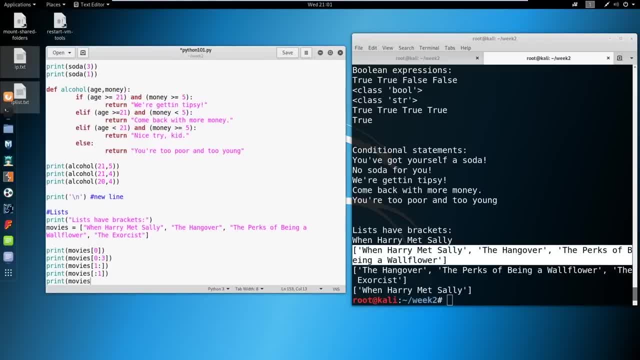 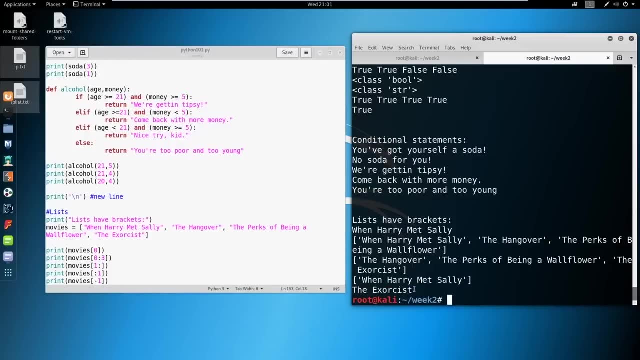 you can name names, but snitches get stitches. just remember that. snitches get stitches. all right, let's check the negative one out. pulls out the exorcist. so negative one pulls the last item out of the list. okay, and lastly, we can also print the length of this and see how many movies are in this list. here got four movies in list one, two. 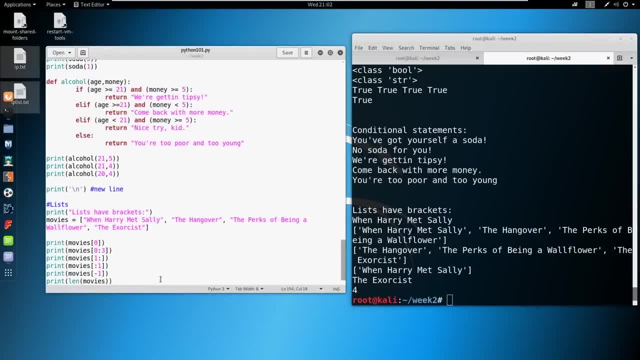 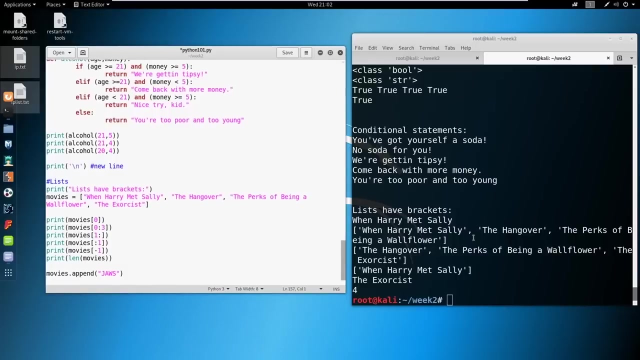 three, four. yeah, that's correct. okay, on to some other tricks. let's say we want to add a movie to this list, say we want to add in jaws, we'll just type movies, dot append jaws. now if we say print movies, where do we think jaws is going to be at beginning, middle and random? yeah, negative one. 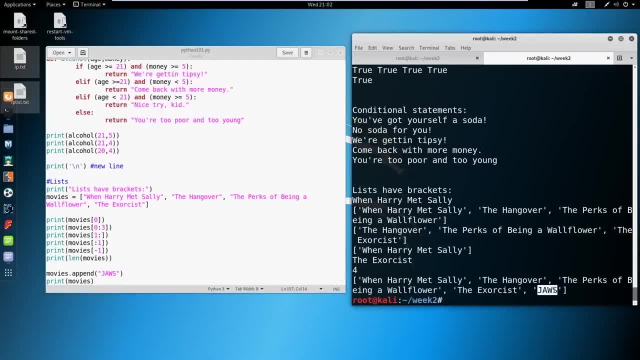 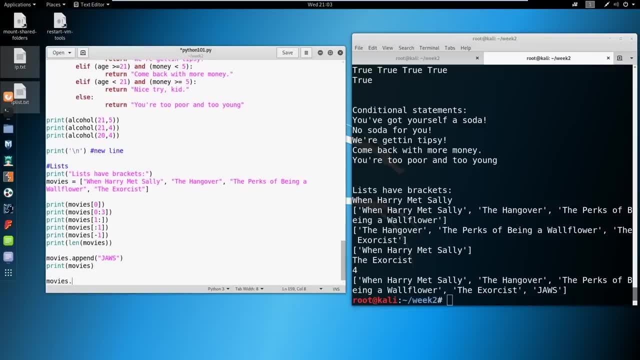 right the end. jaws is now in at the end. okay, what if we wanted to remove? jaws could do this cool little trick called pop. if you don't give any number to pop, pop just removes the last item in the list. so if we pop this list here and we say print movies. 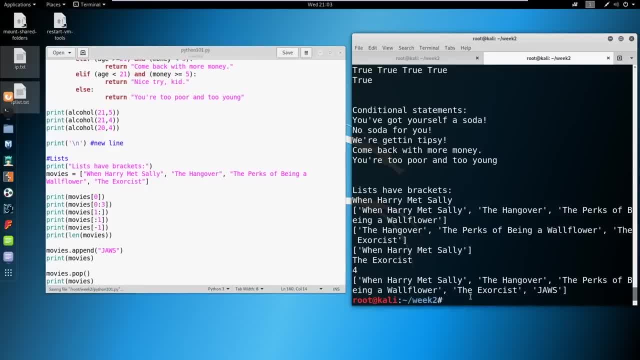 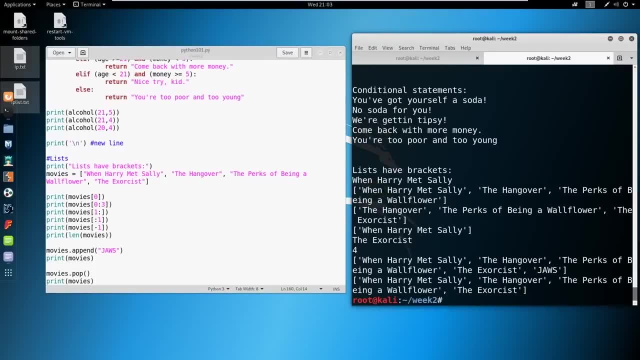 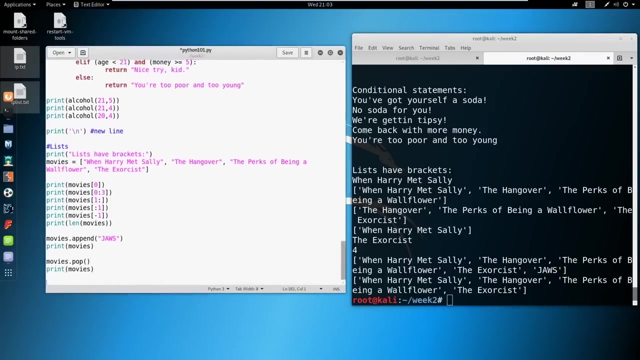 okay, try it again. you'll see that jaws is now gone. okay, we've got a food theme going: white rose, it's all right. all right, let's say we wanted to remove a specific item let's get rid of. uh, we'll get rid of the hangover. let's say it was the hangover three. 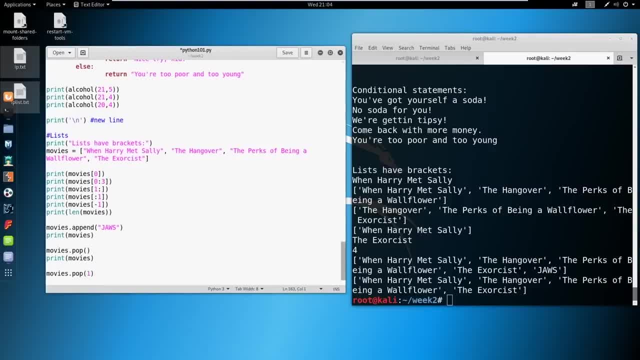 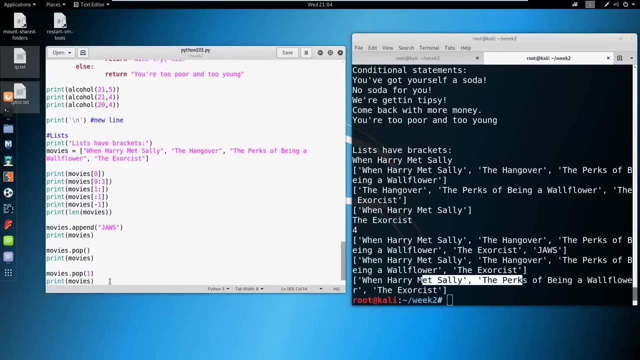 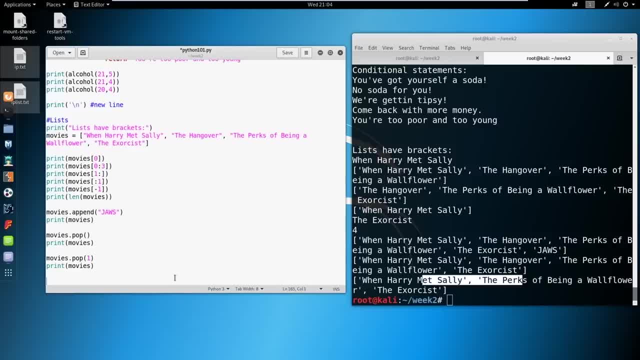 let's take a look at that. i'm going to copy paste this whole thing again. just keep the same list and let's add to this another list. let's say, for person, let's say that my favorite movie is when harry met sally and i don't know. we'll say jake likes the hangover. 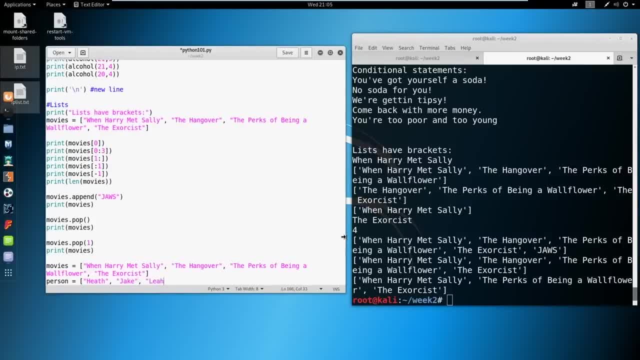 and leah likes perks of being a wallflower because she's british and loves emma watson, and we know jeff likes the exorcist. so we'll do that, okay. so now let's say we want to combine these two together. let's say we want to pair it up. 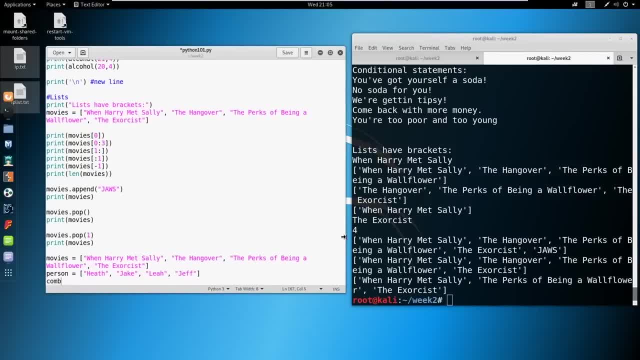 just the way. it is okay, let's call another variable, we'll call it combine. we can do something called zip. we say zip movies person, and then we're going to print it out as a list combine. so zip is storing it into memory. i believe is how that works, and then you put it down into a list. 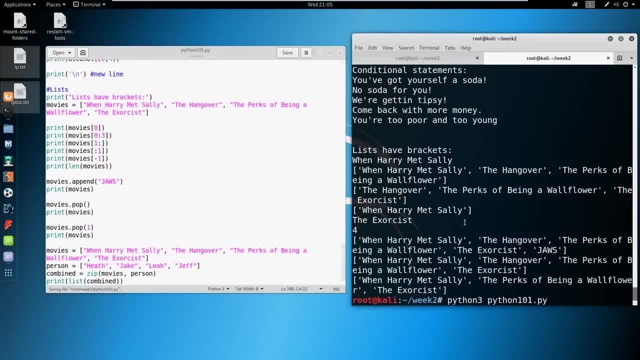 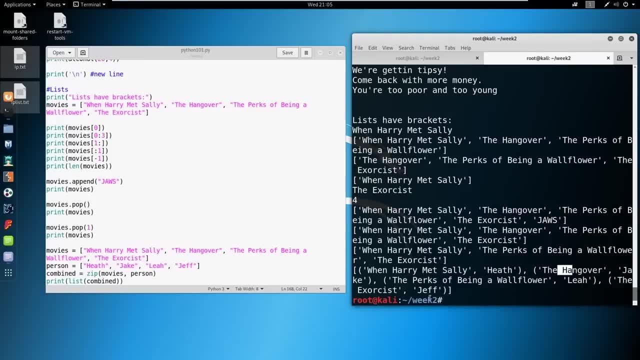 and we print the list and you can see that. okay, i like this movie. jake likes the hangover, leah likes the perks of being a wallflower and jeff likes the exorcist. yeah, neat little trick, it's list-ception. it is a list in a list. yeah, exactly. 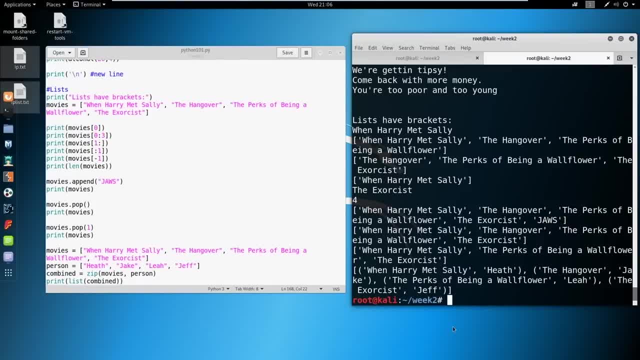 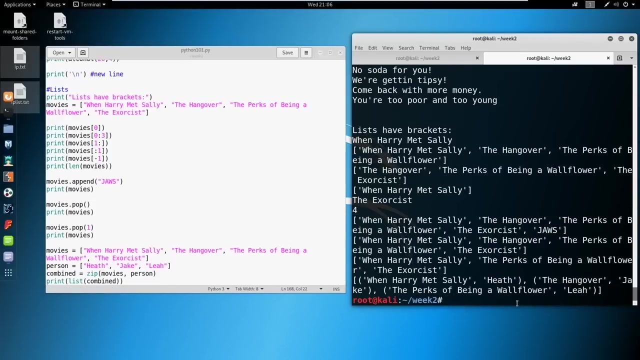 okay, so that's really it for list. what happens if you have four movies but three people? that's a good question. you won't have anything there, let's see. let's just take out jeff. bye, jeff, let's try it again. ah, look, it's just gone. there is no exorcist tied to jeff. there's no exorcist at all. 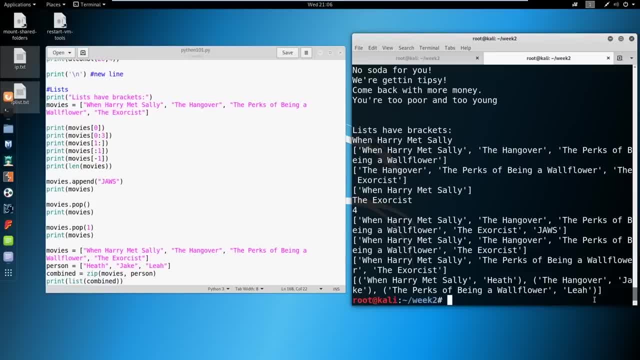 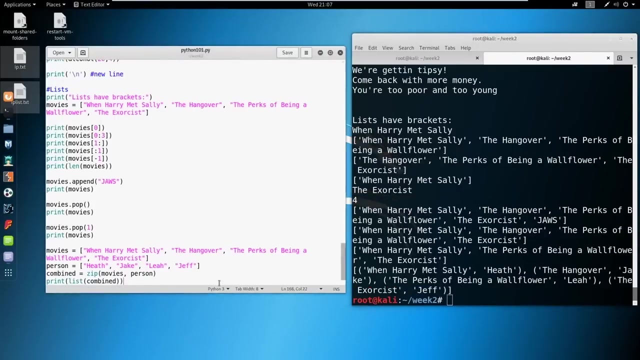 up. i'll add jeff back. there's been been requests for jeff to come back. all right, okay, he's there, let's be happy. okay, somebody just mentioned tuples. we're going to talk about tuples later. we're going to talk about tuples really, really, really, really quick, very quick. We might actually get done early. 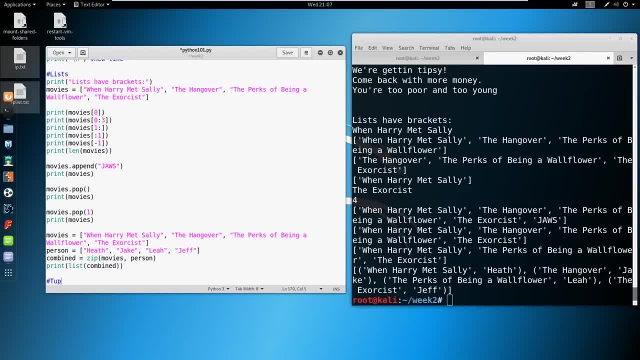 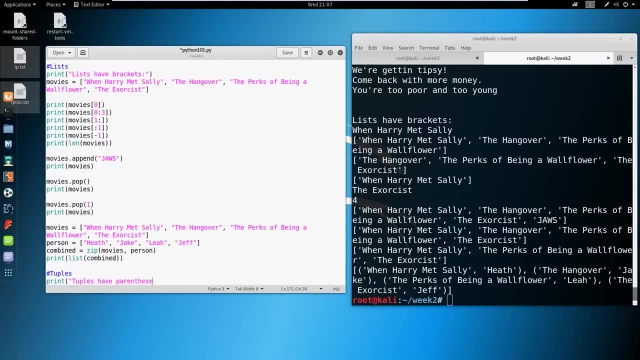 I don't know. Okay, Tuples have parentheses and cannot change. So think of a tuple as a list that cannot be modified. So what's good for that? Let's say, like grades, If we know, grades are always A, B, C, D and F. 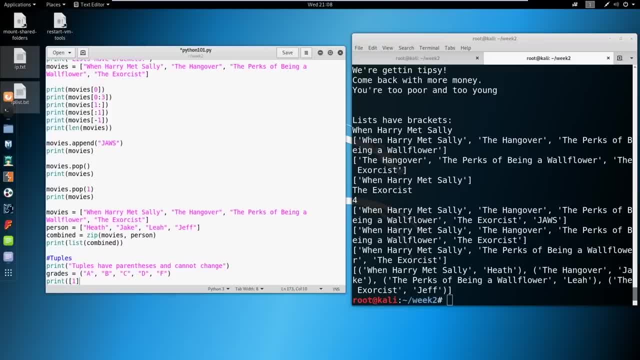 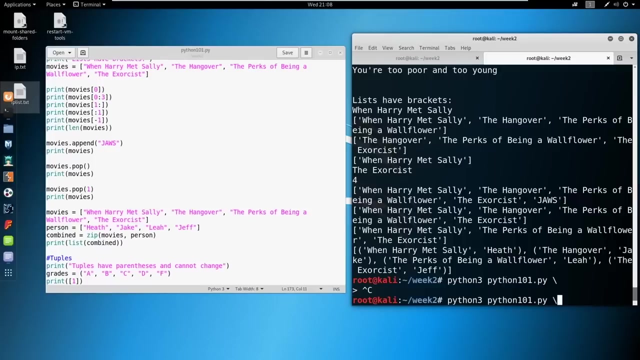 we can print out a grade So similar to before. What are you going on about, Scott? That's too smart for me. Oh, typo. Okay, Tuples have parentheses and cannot change. I did not print the whole tuple because I. 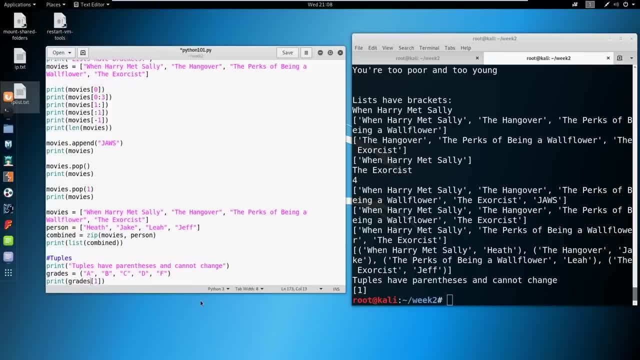 just printed a one out, My B Save. Try it again. All right, We printed B, But we couldn't sit here and pop the tuple. We couldn't append the tuple. The tuple is static. It's a good way to think about it. 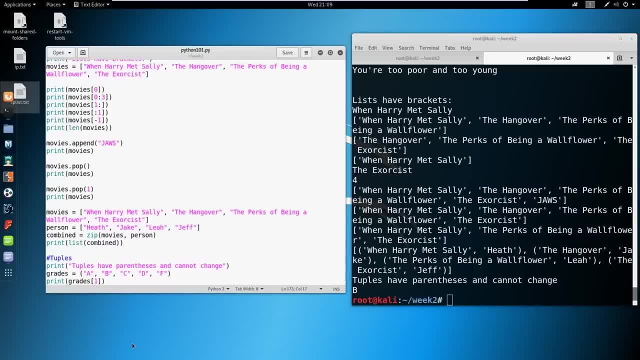 So there are also dictionaries which I don't think we're getting into dictionaries tonight. If we do it next week, we'll cover dictionaries, We'll cover classes. Let's see, We've got looping left and then we're going to cover some code. We'll talk about code. 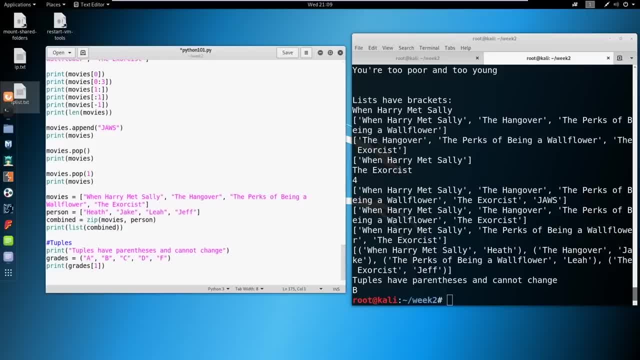 Remind you on the AMA. It looks like the AMA might start early, Okay, Okay. So we're going to be going into looping. Okay, We're going to print for loops start to finish of iterate. It's a good way to think about them. 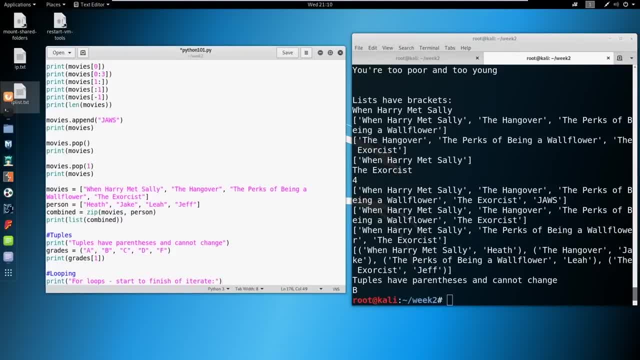 So remember, remember that we were doing for loops last week, right? So we did a for loop when we were going through our IP addresses, Oh, okay. So question on the tuple. The tuple is: why is the tuple a tuple? If you look, the tuples have parentheses. 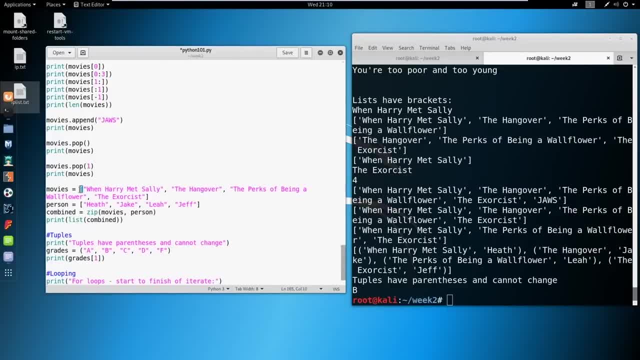 The lists have brackets. The list has brackets. See the bracket. See the parentheses. That is the slight difference. What is the word when they can't be changed? Is it immutable? Is that the correct word? I don't have all my coding language down: Immutable- Yeah, So we're immutable. 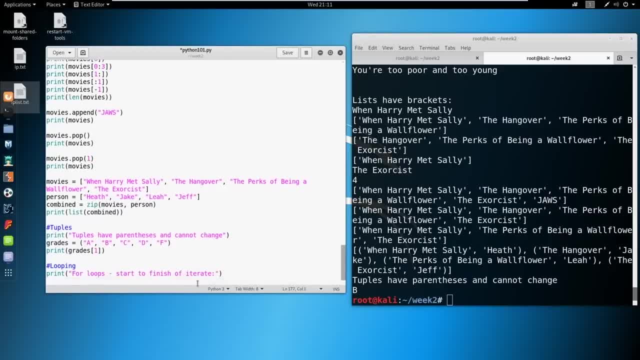 Okay. So when we talk about looping now, we're going to do something like I was talking about last week. Last week was when we looped through our IP address. right, We said, okay, we want to go through a sequence of 1 through 255, and we want to do that until it's done. 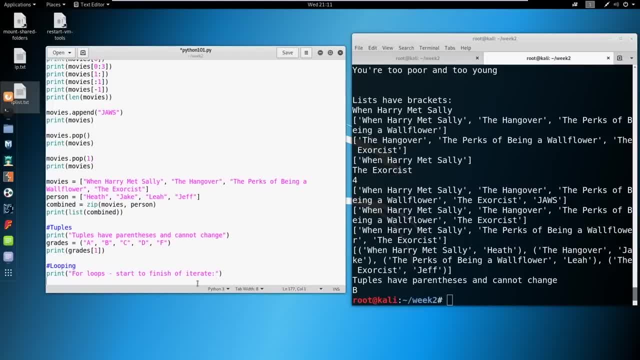 So we had an iterate. The iterate was 1 to 255.. We're going to continue through until we are done. That's really the theory behind the loop. The for loop is through the iterate right. So for 1, for 2, for 3,, for 255, until we finish. then we're done. 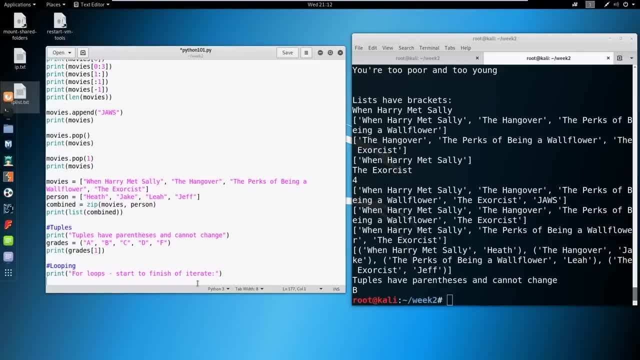 Now there's while loops as well, and while loops are a little bit different And we'll go over both of those and why they're different. So let's look at a for loop again. Let's just declare a list here. We'll declare some vegetables. 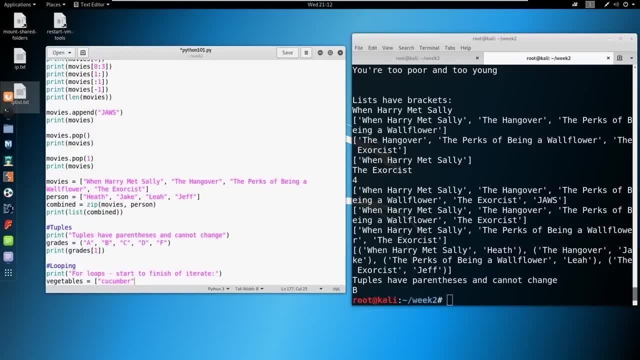 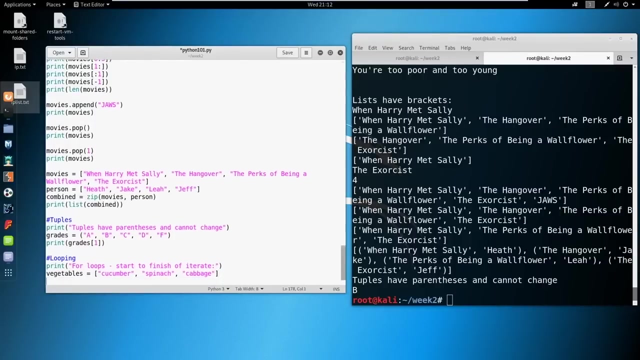 I don't like vegetables, So I don't care what your favorite vegetables are. They're all gross to me. How can I not like vegetables? Pizza is a vegetable. Thank you, I plead the fifth on the vegetables. Okay, All right. 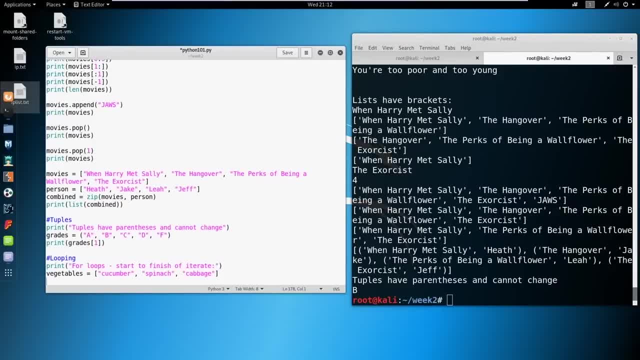 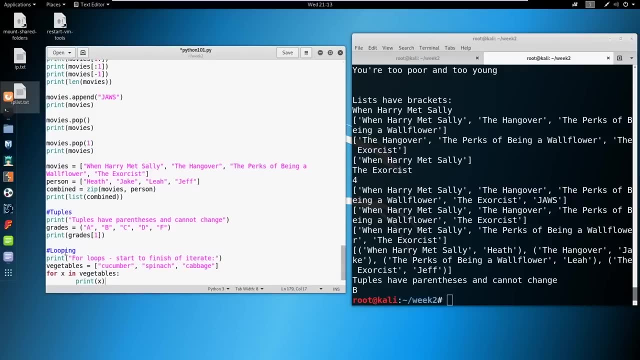 We've got vegetables defined. We could do a quick little loop that says: for x in vegetables, print x. All this is doing is for x, which x's can be. whatever you want to call this, You can call it veggies or whatever. 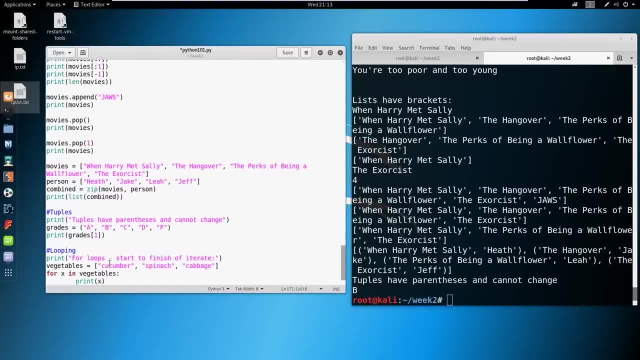 For veggies and vegetables. you print x. All we're going to do is we're going to call it vegetables. All we're going to do is we're going to call it vegetables. All we're going to do is we're going to call it vegetables. 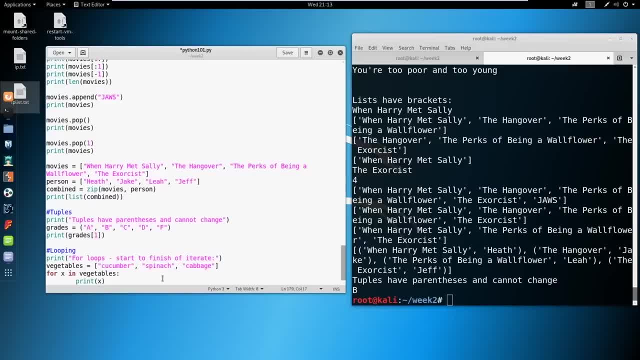 All we're going to do is iterate through this list until we're done, and then we're going to stop iterating A happy little loop. Yeah, We're like Bob Ross here, We have a happy little loop. So remember, last week, same thing. 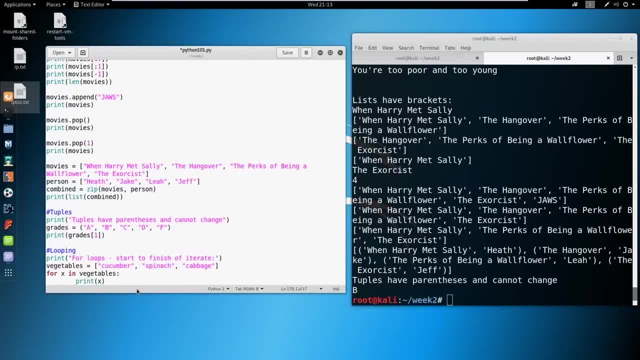 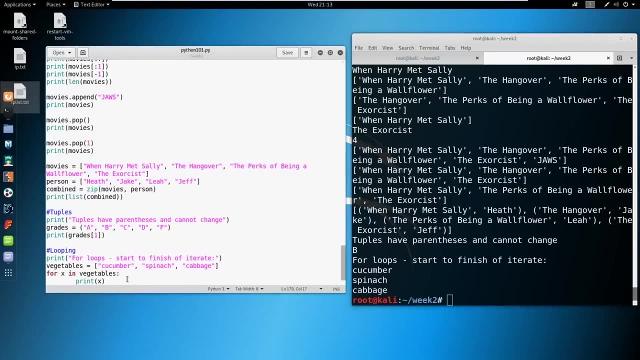 We were for 1 through 255.. As soon as we hit 255, we were done. This is the same concept, So let's go ahead and save this. Okay, You see here cucumber spinach cabbage. Okay, We loop through that. 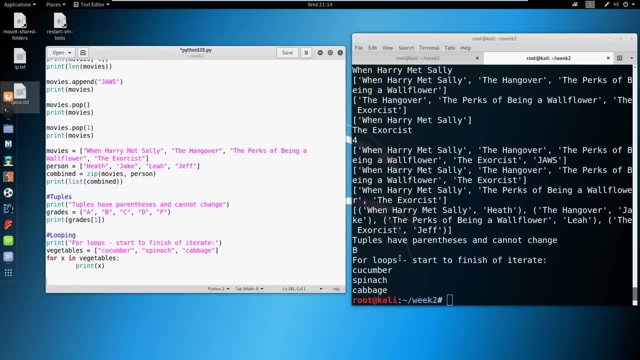 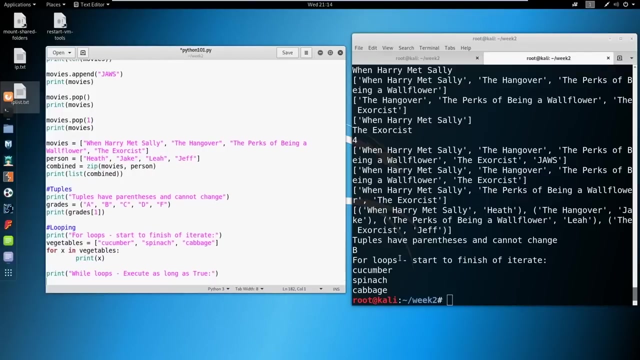 I like hitting the button. It gives me purpose. Leah, All right, Let's talk about while loops. These execute As long as true. Again, remember capitalized D, just trying to emphasize that. Okay, A common way. you're going to see these. 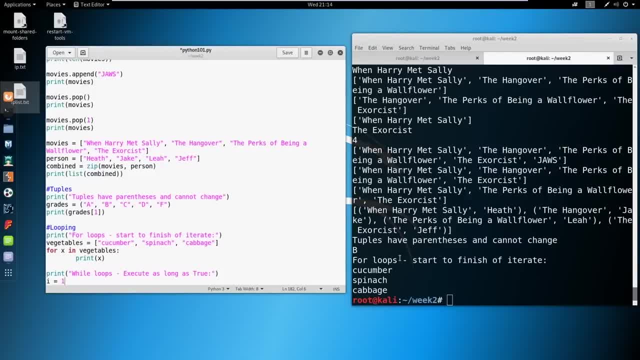 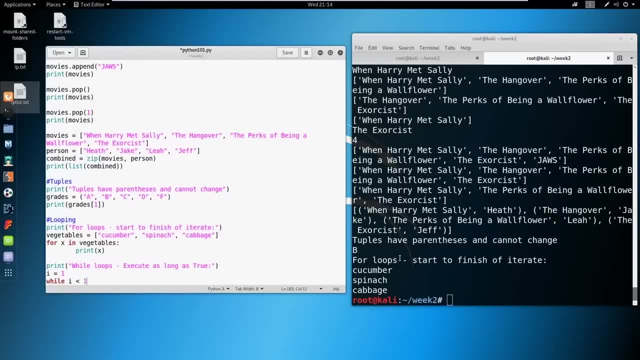 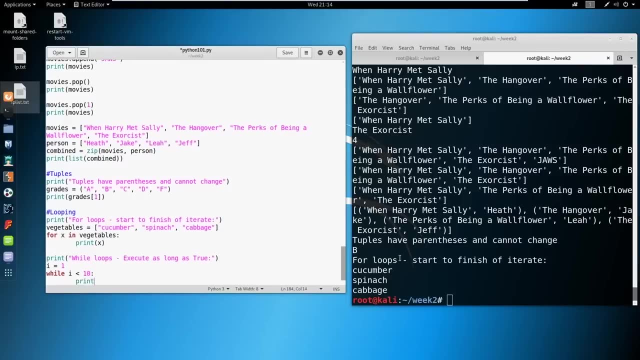 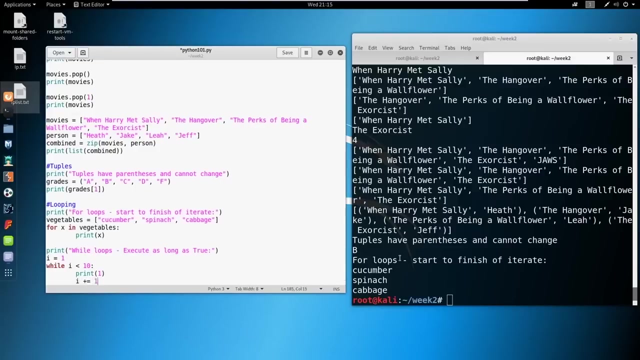 We'll declare I equal to one, And a lot of times you'll see, While I equal to one, Okay, I is, let's just say less than 10.. We'll print I, And on top of that we're going to say I is plus equal to one. 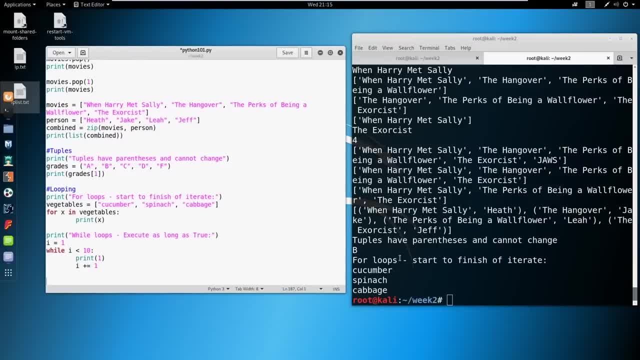 So this is going to count up to 10.. Essentially, We're declaring that I equals one, While I is less than 10, one is less than 10.. We're going to print: I. I put print one. Yeah, Thank you. 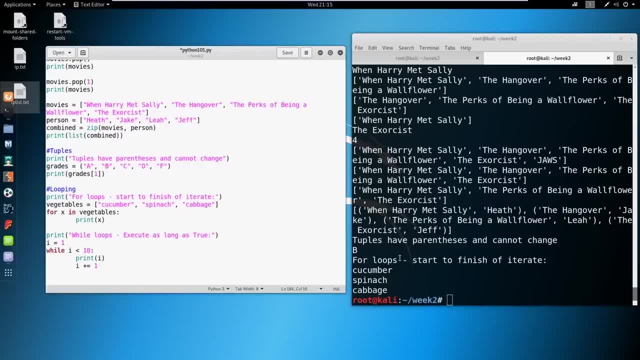 Noticed, print I, And then we're going to do I plus one. So what's going to happen is I is then going to become two all the way till we get to 10.. So all we're saying here is: while true, we're going to do something. 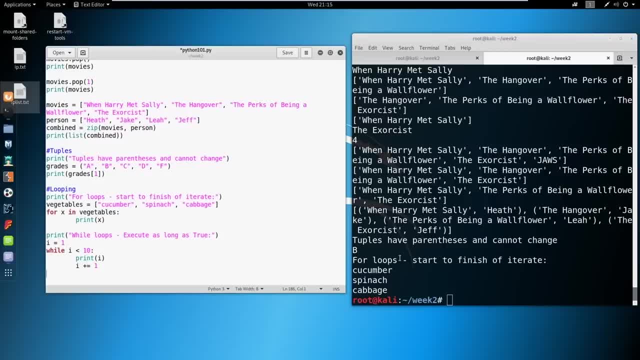 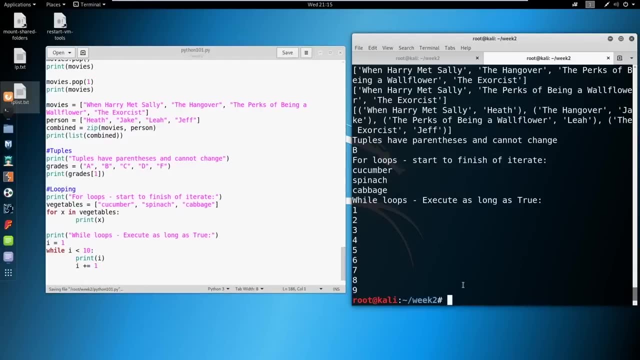 Okay, Okay, So that's it for these We're going to cover now. Okay, here we go. Yeah, it's less than it won't print 10.. You're right, It'll print nine. Yeah, I didn't put the equal sign. 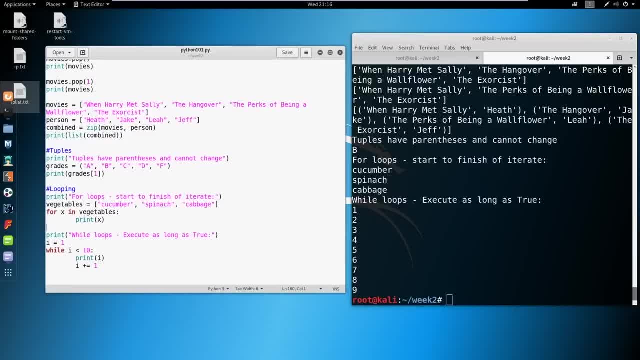 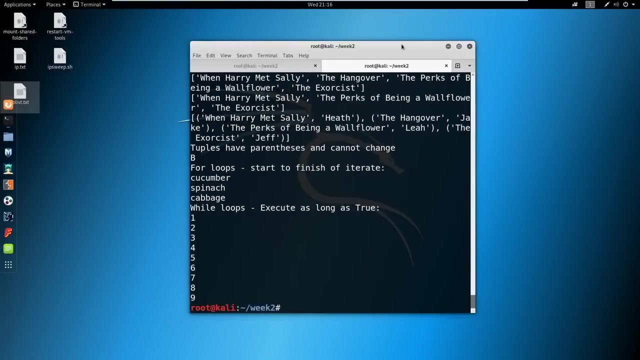 Keep me on my toes. guys, You're like lawyers. You're not my mentees, you're my lawyers. my lois, All right, let's take a look at some code, some other code. Let's save this. So my goal for you is that I want you to be able to read what we're about to see. 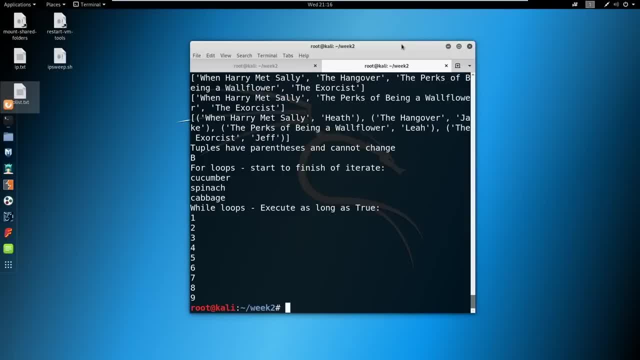 You don't have to understand fully what's going on. You just need to be able to read what you're seeing, in a sense, and get an idea for what the application is doing. There's going to be a lot of things in here that we didn't cover, and that's fine. 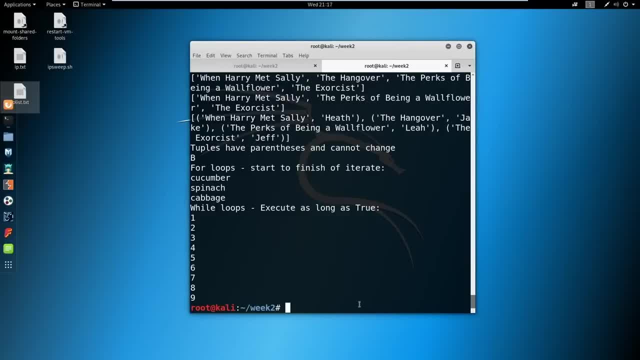 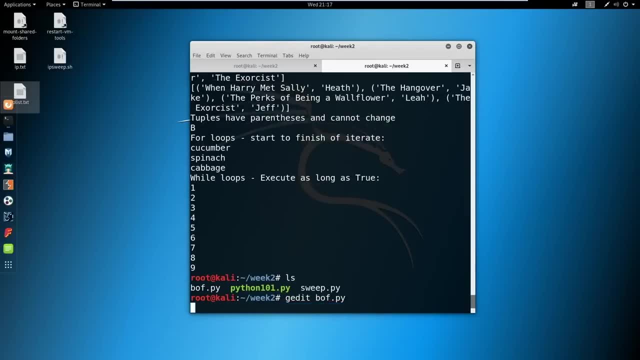 The goal is to be able to understand exactly what you're seeing. So I've got two things in here for us. Okay, let's look at the buffer overflow before. So if you've sat through a buffer overflow lesson of mine, this script might look familiar. 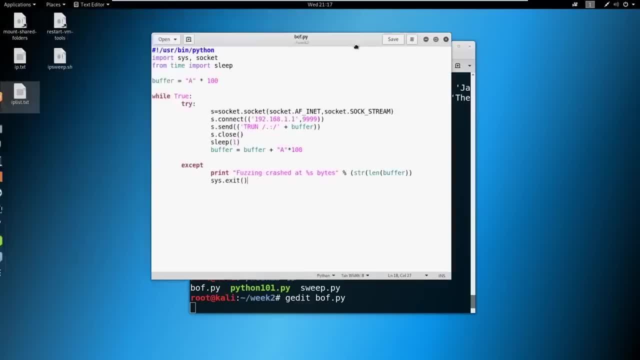 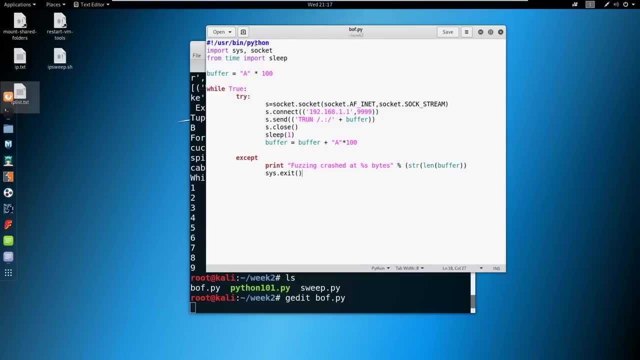 This is a basic, basic fuzzing script. This is written in Python 2.. That's okay, The concepts are still the same. So if we look at this, we're declaring that we're calling out Python here We're importing some stuff. Now, we didn't cover importing, but these are just modules, right? 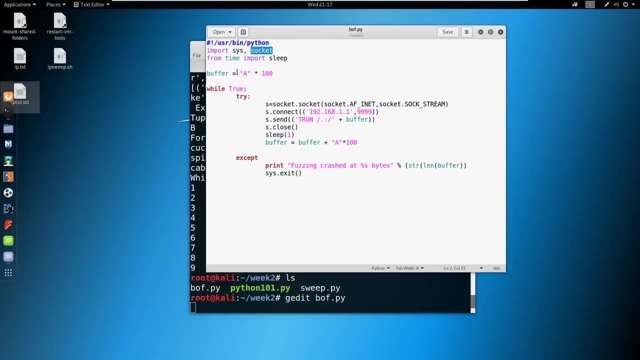 These are modules that we want to import, that we're going to use, that aren't by default sitting in Python itself, but we can import these modules and they'll do things for us. So we've got socket, like the socket module here, that's going to allow us to connect over this socket, and 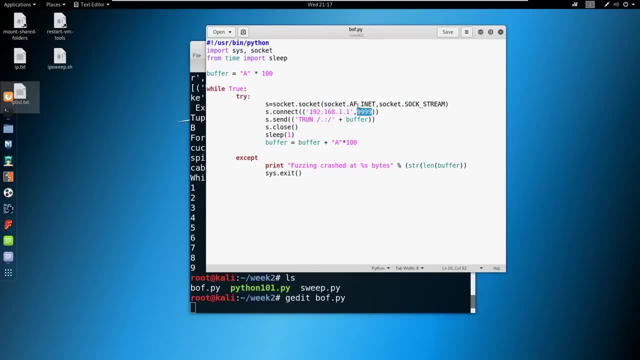 this socket here, which is just IPv4 and a port. Well, I'm declaring it at the top. At the top, that is Python 2.. Yeah, So outside of these imports, let's look at the first line. We've got something that says buffer. It's just a variable right. 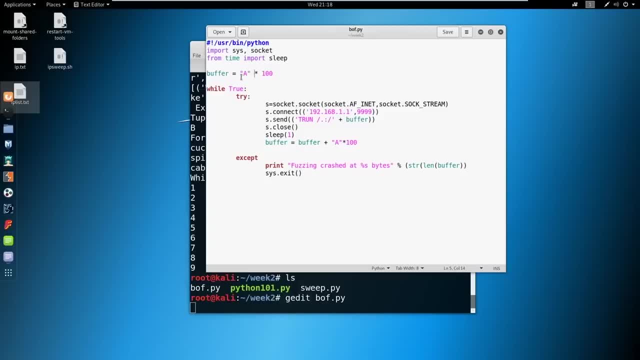 So buffer is equal to 100 A's A times 100.. So this is just a string of 100 A's. Okay, now we've got a wall loop sitting in here. We said wall true. So as long as this is true, this loop is going to run. 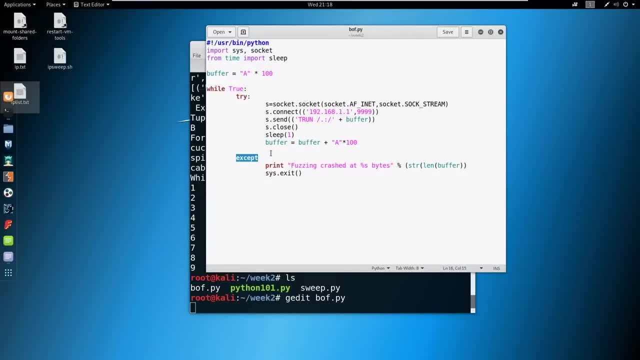 We've got something here called try and accept. We didn't cover those, but you might be able to imagine what they are. So we're trying to do something And if something else happens, then we're going to close out of the program, right? 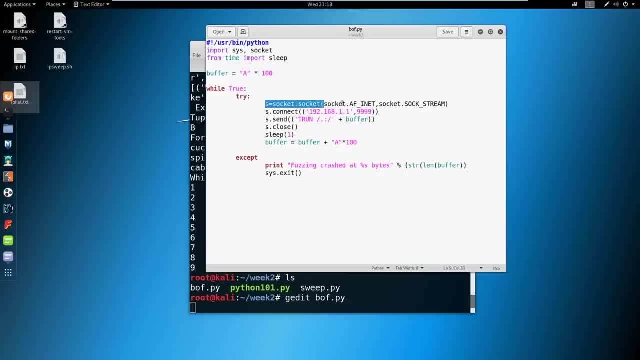 So you can kind of understand already what's going on. So we're actually sending a connection to this IP and this port, We're sending over a message plus that buffer variable here. So we're sending this message plus 100 A's. 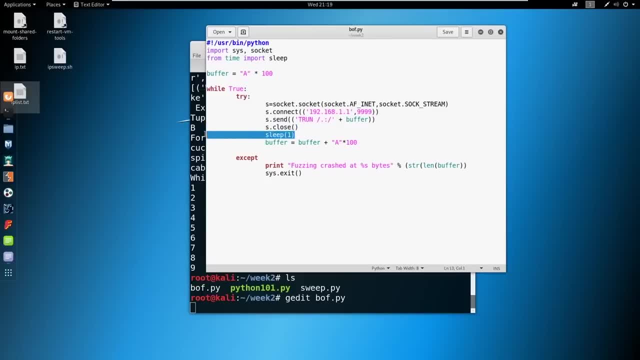 We're going to close out of that connection. We're going to sleep for a second And then we're going to append buffer with another 100 A's, So it's going to become 200 A's And it's going to try this again. 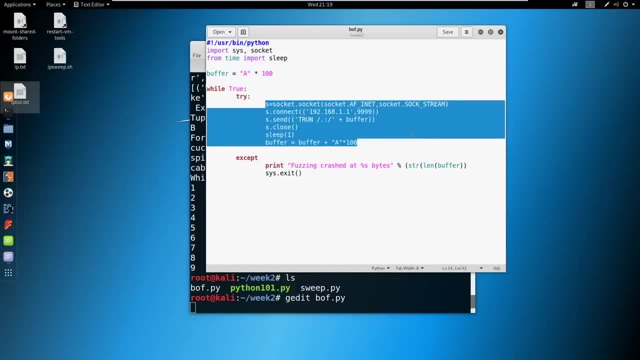 As long as this connection keeps working, this loop will go on forever. All we defined is wall true. Now, if we break this program- which is what fuzzing is anticipating to do- then okay, we're going to say, hey, we crashed it. 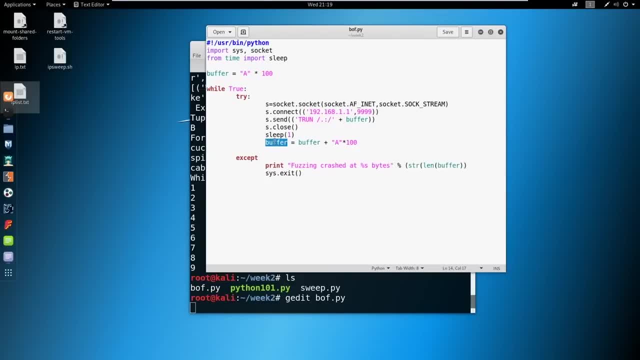 We'll print out where we crashed it, where buffer was sitting, in terms of bytes, And then we'll say, okay, sysexit, close out. And then we'll be done with this loop. I did miss the colon, Good job. 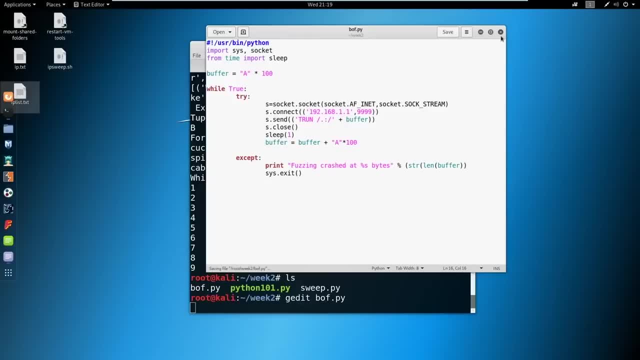 I typed that up today, So, thank you. We're not running it, So, but hopefully this makes sense. This is just like a basic, So we're going to print out where we crashed it, So, for example. I'm going to show you another example here in a second of a more detailed script. 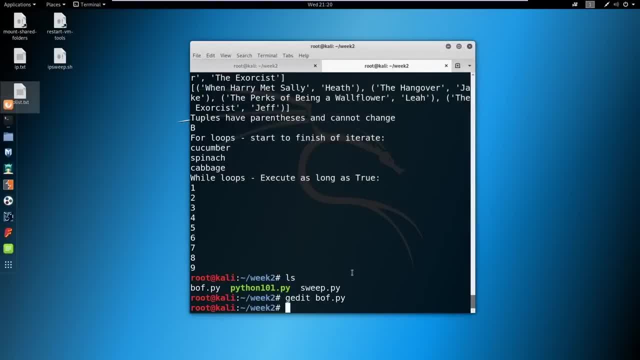 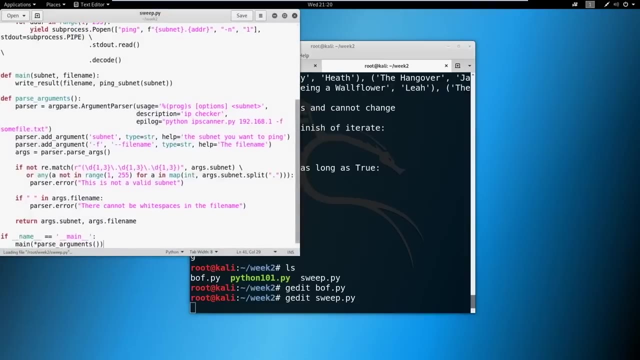 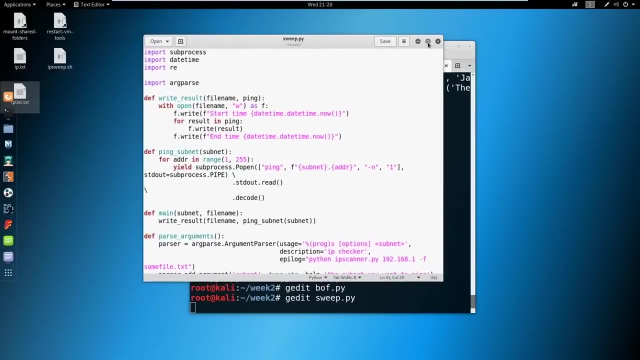 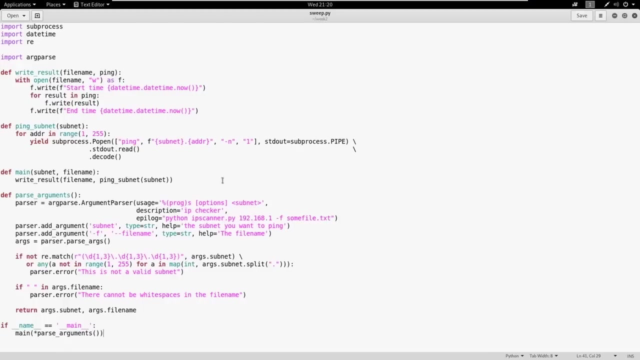 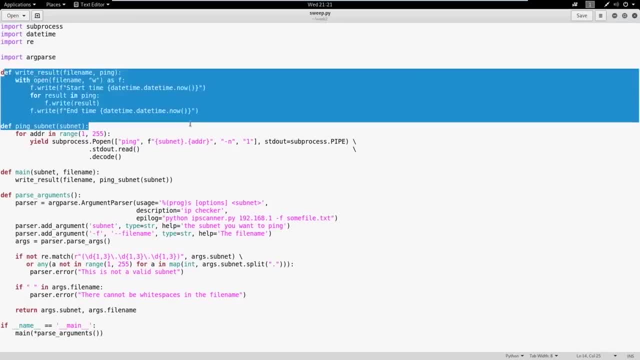 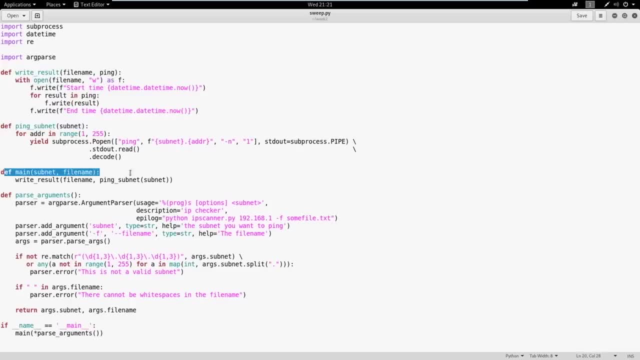 defining a function called ping, subnet, a function called main, which is common parse argument. and then you have this: if name equals main here, This is very, very common as well. So what we're looking at, we see that some things have been imported. 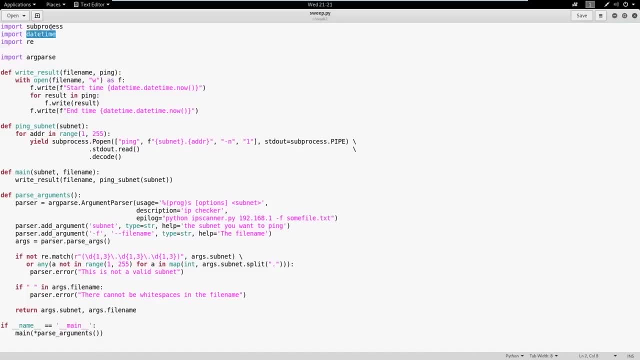 You don't have to know what these are. DateTime is kind of obvious. SubProcess, I believe, is for files. argParse that's for arguments, so like if you have a switch, like when you type in dash, dash help. that's for arguments, and you'll kind of figure that out here in a second. 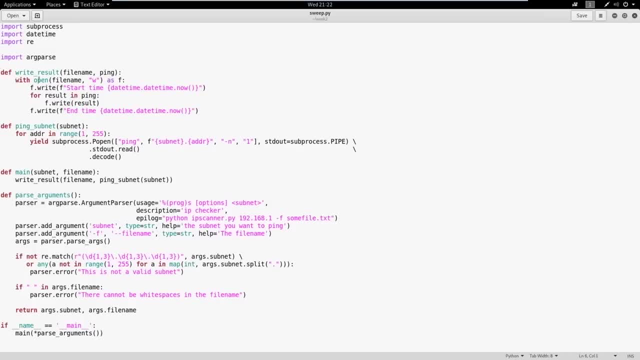 So let's look at the first function and just see what it's doing. So you see it's defining writeResult with file name and ping. So it looks to me as if this is writing out a file. So it has declaring as f f, dot, write, okay, start time. it's. 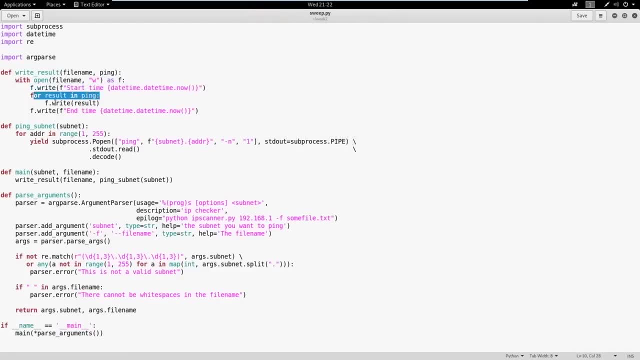 giving a date time now For result in ping. it's gonna write to this file the result and then it's gonna write the end time. So you don't have to know how to code this, you just have to be able to know how to read this. Okay, let's look at. 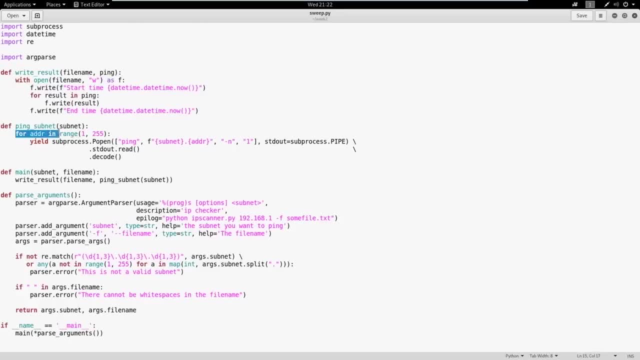 ping subnet For address in range 1 through 255. that looks familiar, right, We're gonna yield the subprocess with poppin. all poppin does is start a process. This is going to ping the subnet, the address that we defined here right- 1 through 255, and it's gonna give it a number of 1.. So 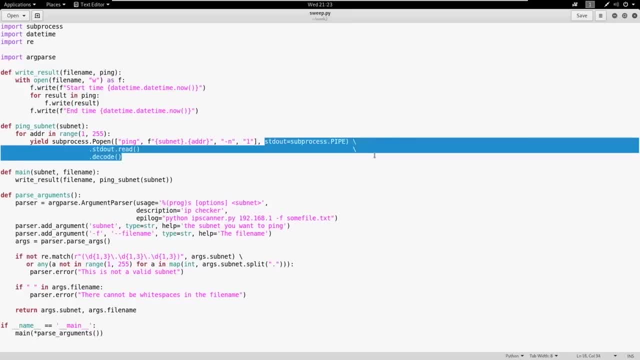 we're pinging one time and then it's got some some information here. don't really need to know what that's doing either. Okay, we're defining our main function and down here we have parse arguments. So this is where this arg parse comes into. 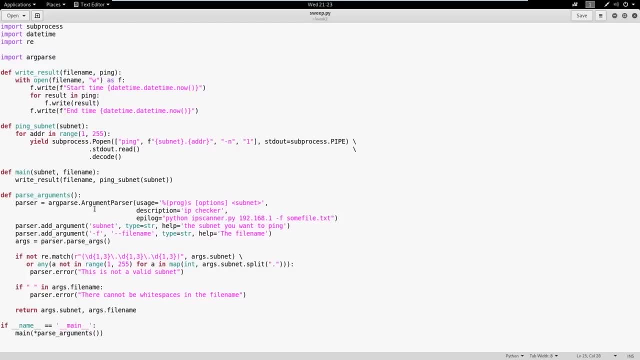 play. If you look through here you can kind of make out what it's saying. Okay, so it's giving you a description. it's an IP checker. it gives you the usage, the epilogues at the end, just giving you the how to run the syntax. So it says Python. 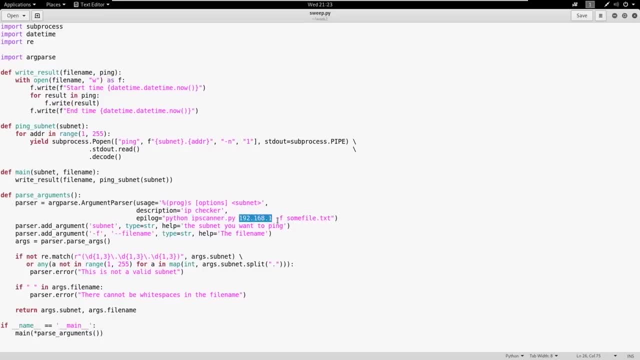 IP scanner, dot PI 192.168.1, and then a dash F to save to a file. What if the subnets not slash 24? then this script won't work for you. This is a very basic script. You're probably not writing your own ping sweeper anyway You. 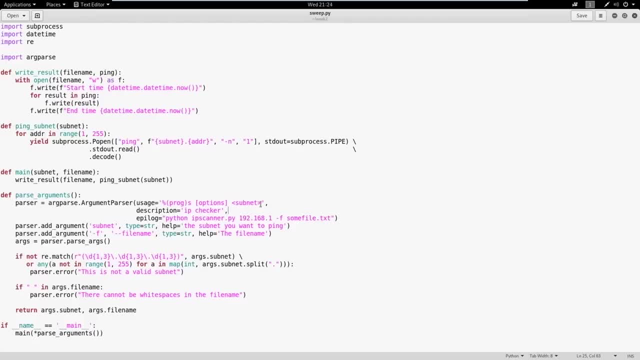 could write it a lot faster in bash. This is just a good practice one, Okay, and then. so you've got your parser add argument. So it's got a subnet argument. It's got this dash F or dash dash, file name argument for the file name. 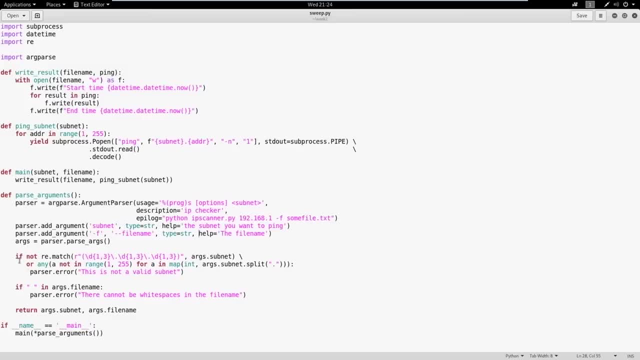 And then you've got these statements in here where, if you don't have your subnet is what it looks like, or it's not in the range of 1 through 255, then it's gonna say you're not in a valid subnet. So it's looking that. 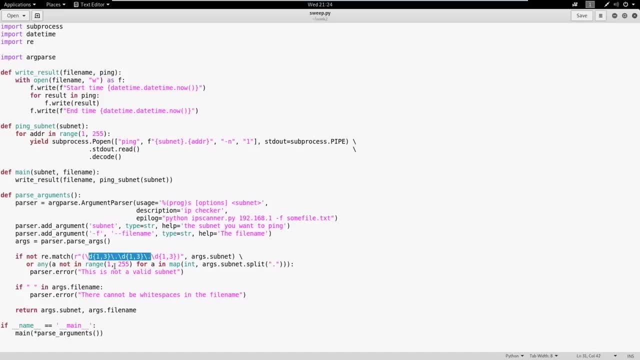 these have three numbers, right, and or 1 to 3 numbers, I should say, and that the numbers are between 1 and 255, and it'll say, okay, this is not a valid subnet if you don't have it correct. And then there are no white spaces that could be in the 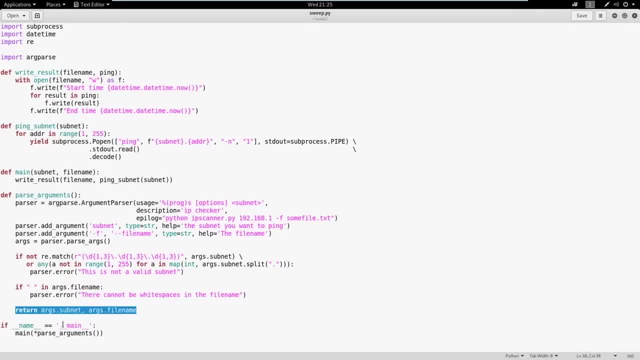 file name. Other than that, it's going to return the argument subnet argument, file name, And then this is just a safety measure here. So that's really it. You don't need to know exactly, as a junior-level pen tester, how to write this. You need to be able to look at code like this and say, okay, I can kind of. 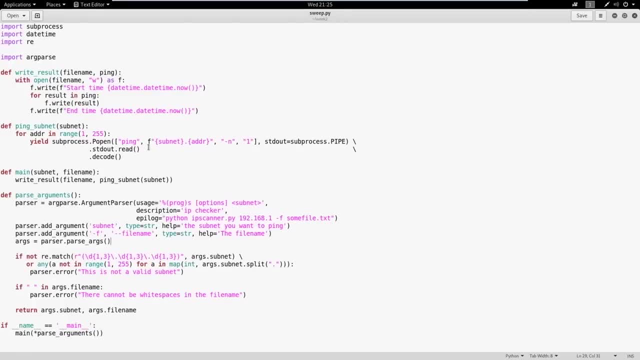 read it and understand what's going on. I might not know everything that's inside of there. There might be some things that I need to Google or look up, but for the most part, the concepts are there, the concepts that we talked about. you see a function. the other one. you saw loop. you see a for loop right here. you see a. 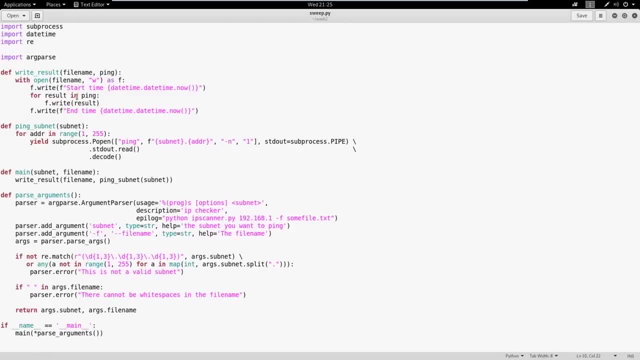 for-loop right here And you're off. Ingredients are that I'm VO log a operator right here. You're understanding what these things are. You see a conditional statement here with the if right You see or you see not. So these things are commonplace And my goal tonight was to teach. 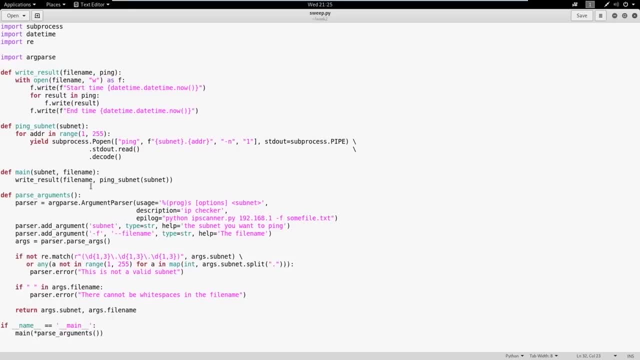 you the commonplace. My goal wasn't to make you some super coder or make you, you know, I don't know well versed, but just enough to be able to get by, If you put in the time over the week or if you want to put in time later, with the course I sent out on Codecademy and the one 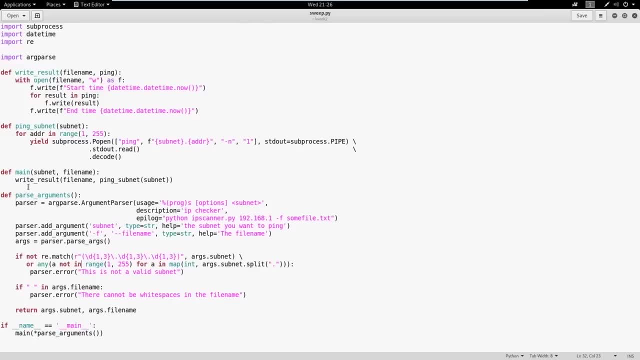 from Cyberary. those are fantastic. Like I said at the beginning of the stream, if you weren't here, I only used the Cyberary course prep for my OSCP. I didn't use anything else. That was all I needed. Got through my OSCP no problem. A lot of the OSCP is just finding code like this and swapping out. 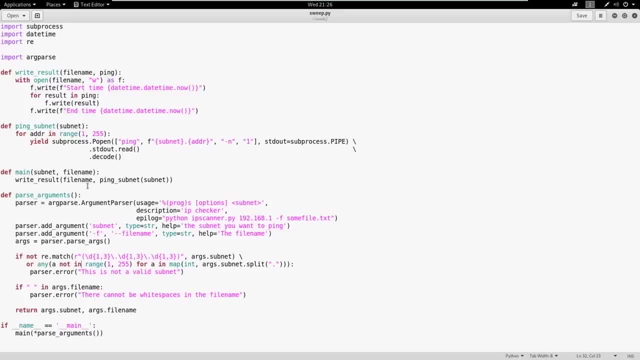 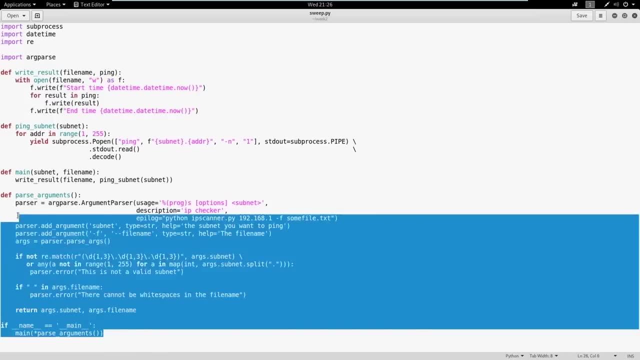 what you need and being able to read and understand what you're doing. Sometimes you will run into code on exploitdb that is broken. You'll have to put that through an IDE or understand where the sometimes. I've seen spaces wrong for Python code and I've just 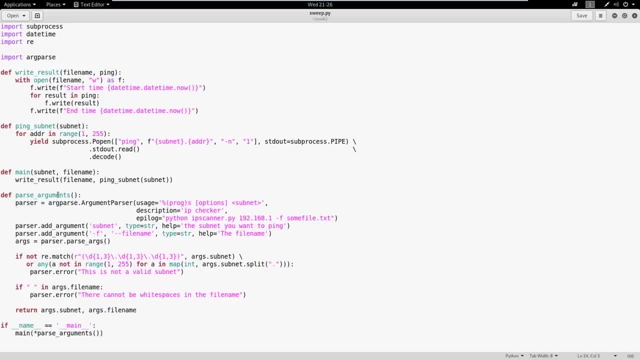 had issues with code before off of exploitdb. So you just have to kind of understand what you're looking at. that spacing is important, what some of these functions are and these tools are. So that's really really it. I actually finished a little bit earlier. 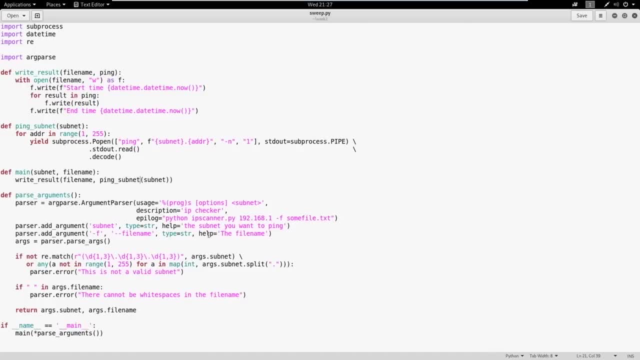 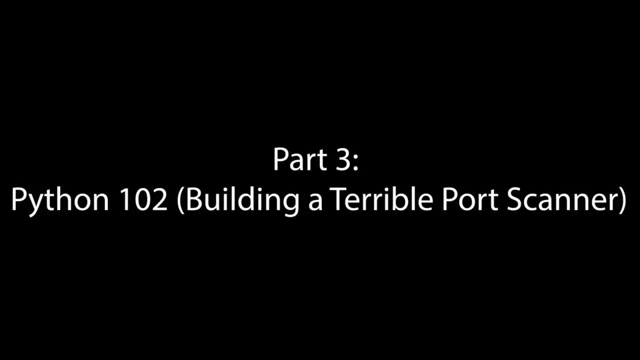 I'll put up my poll. If you guys want to do another round of Python next week, we absolutely can do Python again next week. If not, we're going to dive right into pen testing. We're going to start with the procedure, the methodology, All right. so we got a pretty chill night tonight. I don't 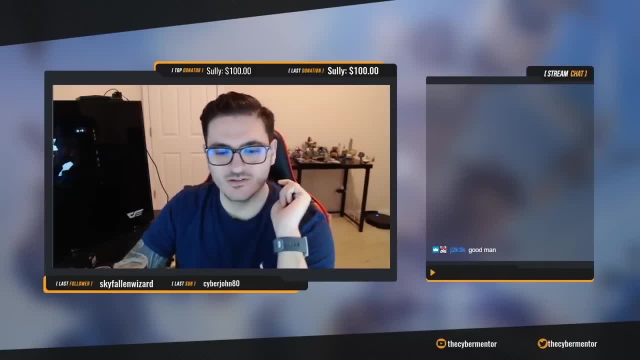 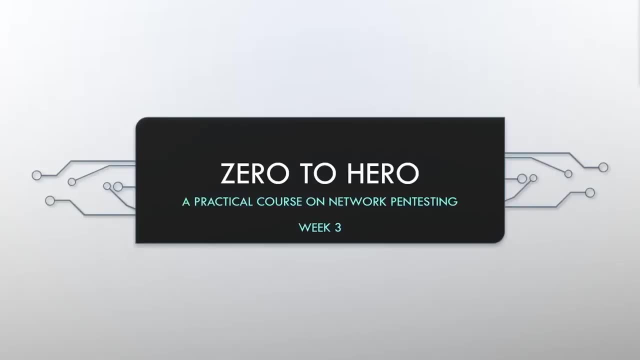 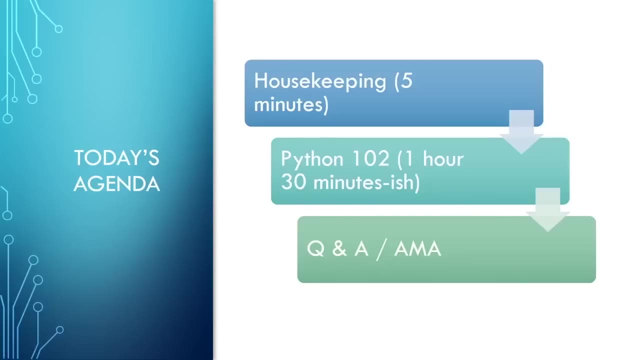 think we're going to be working too hard. I'm going to go ahead and get our screen share here, So we're going to be doing housekeeping, five minutes or so, Python 102,, since you guys asked for another Python lesson- And then we'll do Q&A, AMA, as always in terms of the housekeeping. 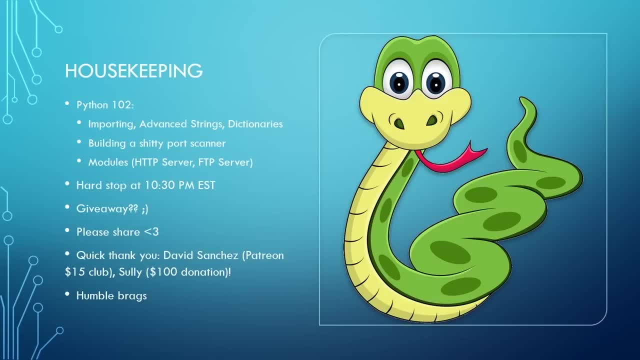 So we are doing Python 102.. As I said, we're going to be covering, importing some of the things that we're going to be doing, and then we're going to be doing some of the advanced strings and dictionaries. Then we're going to build a shitty port scanner. 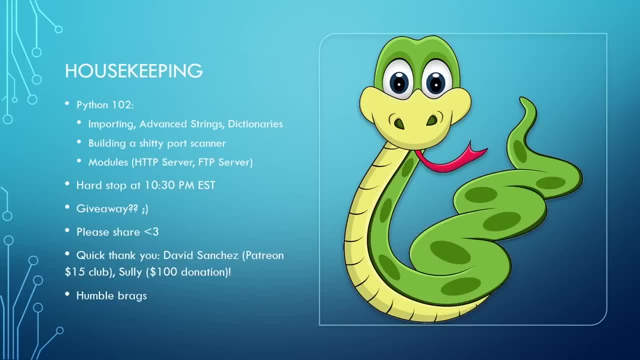 After that we'll talk a little bit about modules. We're going to work on HTTP server and FTP server. We've got a hard stop tonight at 10.30 pm Eastern time, so about two and a half hours into the stream. I have had two hours of sleep today and I am going on a plane tomorrow morning. 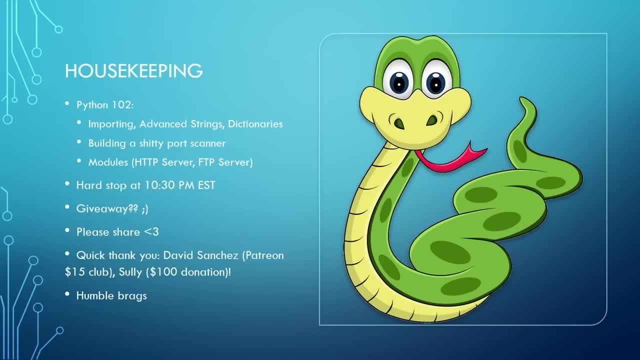 So I need some sleep before I take a little mini vacation here for the next few days. So a hard stop at 10.30. We are also going to be doing a giveaway tonight, So I have next to me a packet squirrel book and a packet squirrel. So I will come back on screen for a second. 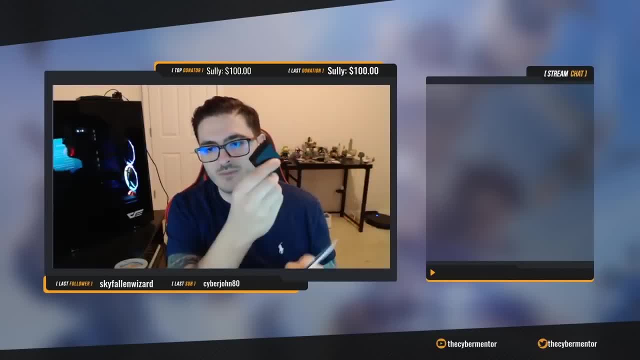 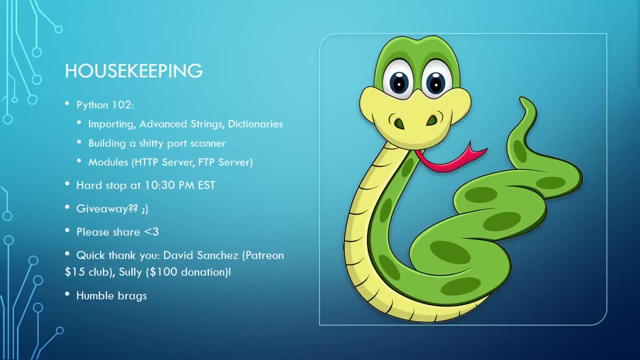 Got the book, got the packet- squirrel, It is yours if you win it in the raffle. This is what we have been waiting for all this time. Let me show you on the screen, just so everybody is clear on how the raffle is going to work. So what we're going to do is let me pull this up. Okay, we're going. 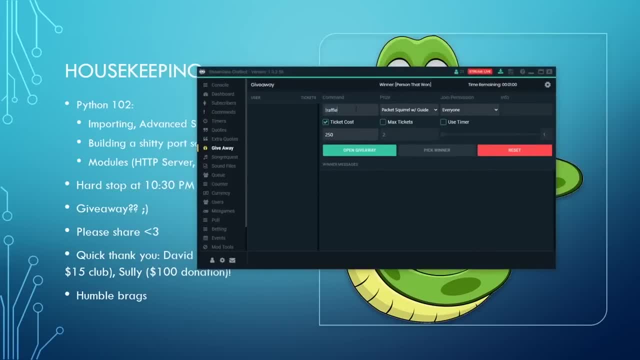 to do exclamation raffle and then you enter the number of tickets you want. So if you want five tickets, you say space five. I can't enter that, but it'll be a space And the tickets are going to cost 250 points a piece. So if you want to purchase multiple tickets, 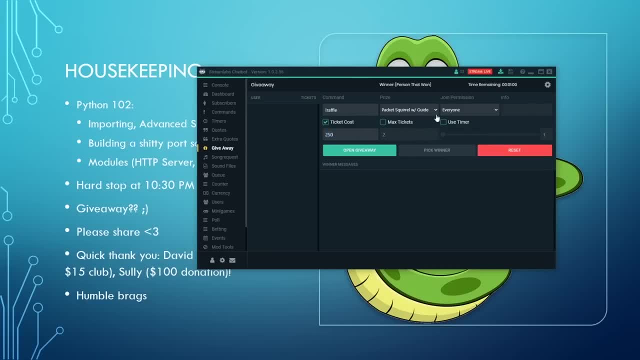 just know how much currency you have and what you can purchase. I'll run a timer, probably for we'll say three minutes. Let everybody get into it, and then I'll open it up and it'll pick a winner at random. 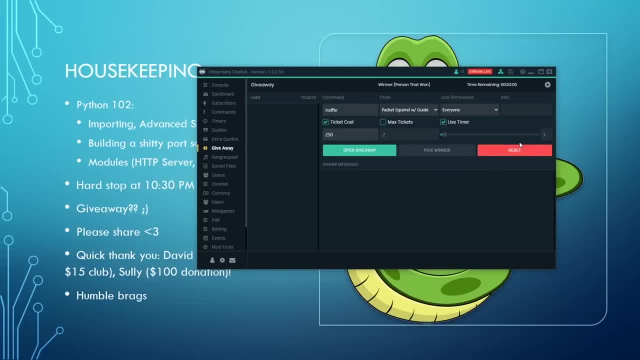 So pretty straightforward. If you want the packet squirrel, do know that you have to send me an address that I can ship it to. So please keep that in mind. I will be hitting you up after this and you will have to give me an address. So anyway, other than that, a couple notes here. 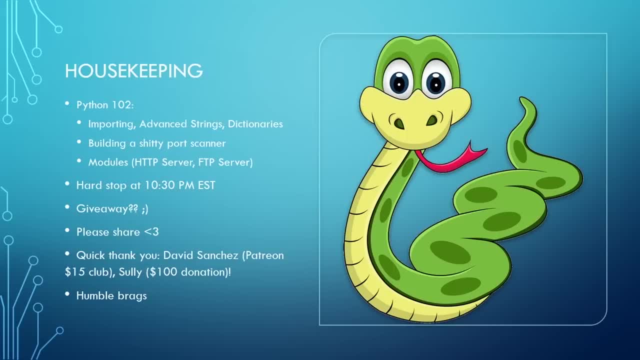 One is: Please share the course if you are enjoying it. Just word of mouth helps us grow, So if you like the course, please just tell a friend or mention on Twitter or whatever social media you're on, and just tell the community, Because the more we grow, the more that I have the opportunity to do. 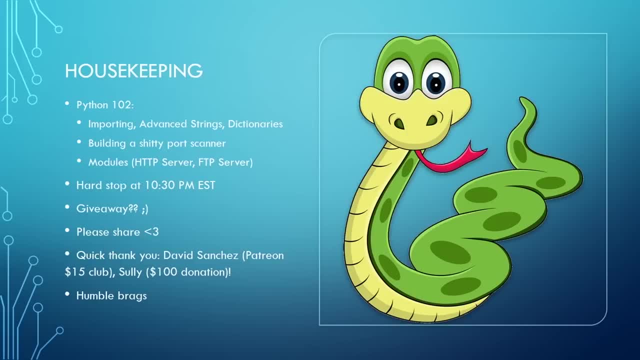 this and teach more often, maybe even more than just Wednesday nights. So that'll be the goal in the long run. So if you enjoy it, please do share. A quick shout out to David Sanchez for joining the Patreon $15 club. Thank you so much for your. 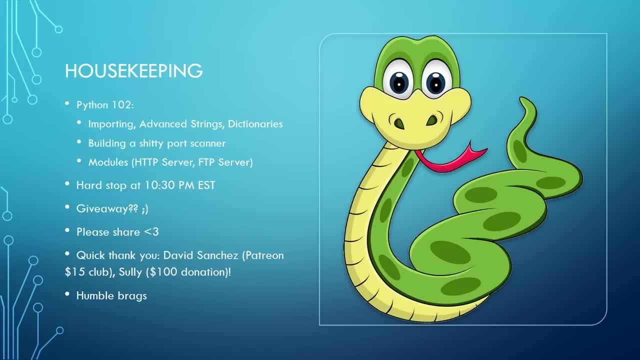 monthly donation And thanks to Sully for a $100 donation last time. I'm not sure that I mentioned it, so I did want to mention it here. Thank you guys. You guys are awesome. And lastly, I've got a humble brag. It's not really a brag, It's just a pen testing lesson, of sorts. So 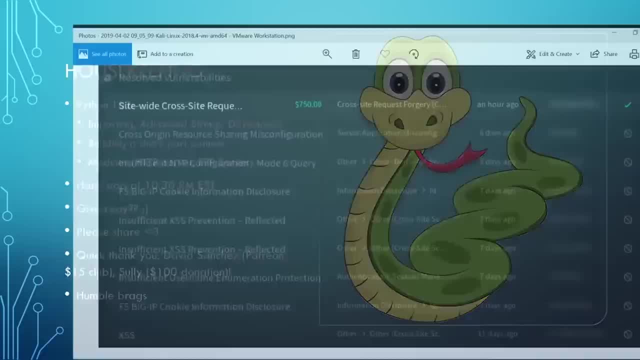 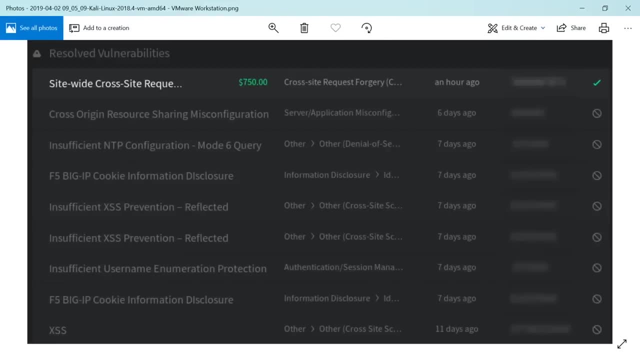 you may have seen this going around on Twitter or LinkedIn, where I got a vulnerability through a bug bounty the other morning. It was yesterday morning or two mornings ago now And if you look where you see the green checkmark you can see all the circled out. 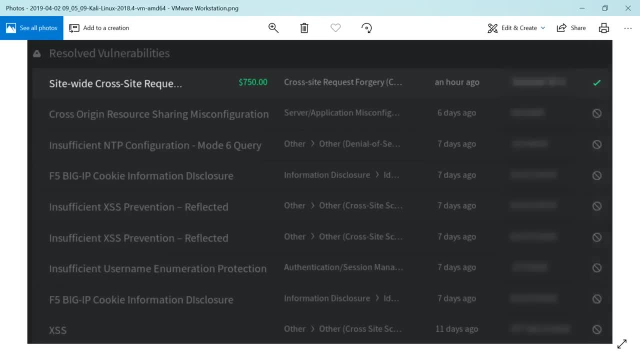 not goods. There's eight of them And really this is kind of what it's like to be a pen tester. This is kind of why I wanted to show this. The first eight vulnerabilities that I submitted were all declined or just turned down, You know. 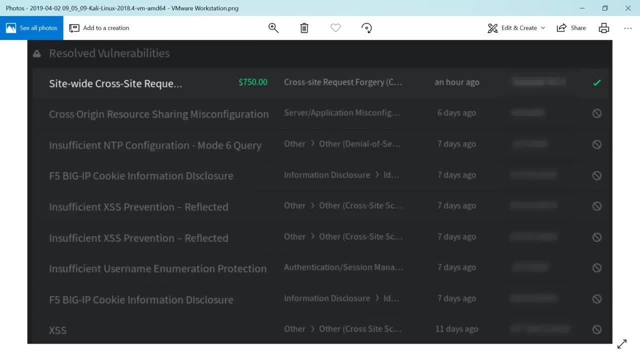 they were not good enough, for whatever reason, or they were too low scope. Whatever the reason was, they got declined. So on the ninth attempt, I finally succeeded, And that's kind of what pen testing is like. This is what: if you enjoy overcoming an obstacle, persevering, you're. going to really enjoy pen testing. So it's definitely for people. you know, if you're a pen tester, you're going to really enjoy pen testing. So it's definitely for people. So it's definitely for people. you know, if you're a pen tester, you're going to really enjoy pen testing. So it's definitely for people. 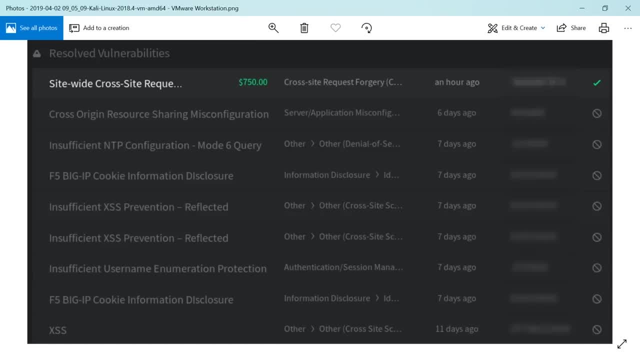 you know they say try harder. I hate saying that, But it really is that. that mentality is that you have to keep going. If you're going to stop at the first rejection or the seventh or eighth rejection, this might not be the field for you. So something to think about If you are. 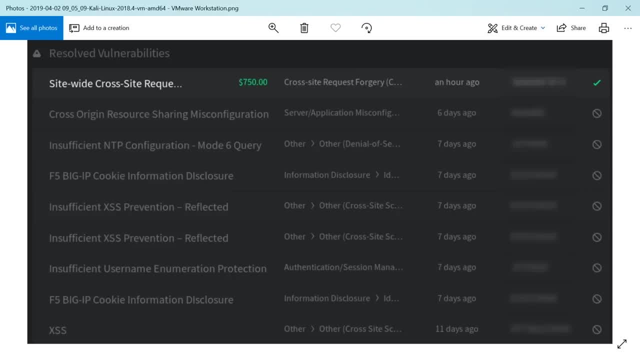 a person who is easily overwhelmed, this might not be the field for you. For those of you that you know, look, I started my first submission 11 days before I got the other one And I submitted, you know, for at least a week, and then hunted that bug down And I 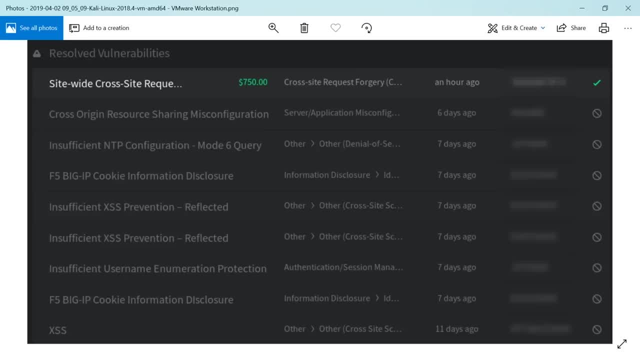 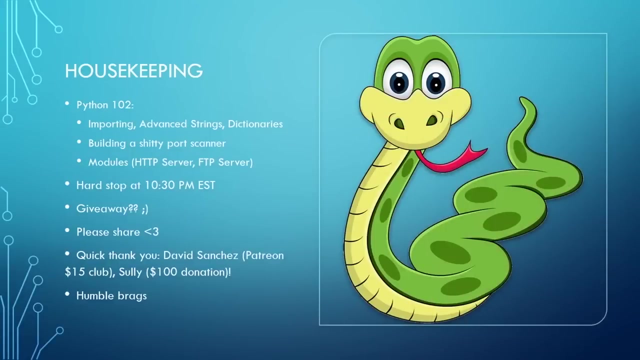 found a bug that I had and I was able to get it down for a week before I found it. So just think about that in terms of doing a penetration test and looking for openings. they're not always going to be wide open. So, other than that, we are ready to dive right in today. Thank you, Cool dad, for. 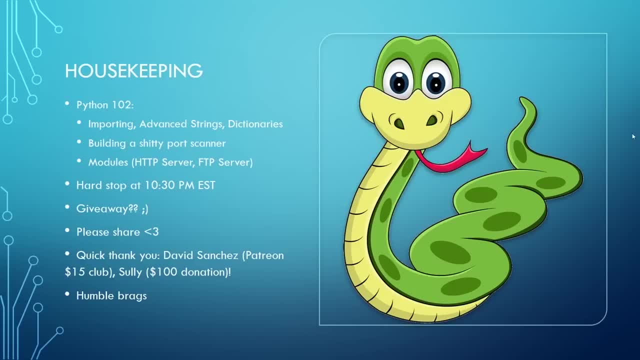 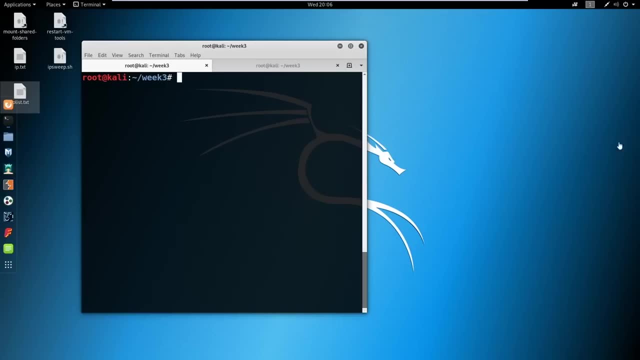 the sub. I appreciate that. Welcome everybody who's joined. looks like we're getting some late comers here. Sorry, I did start the stream a little on time. Usually I started early so we didn't get mistake, Apologize. I was working on getting categories set up which got deleted for some. 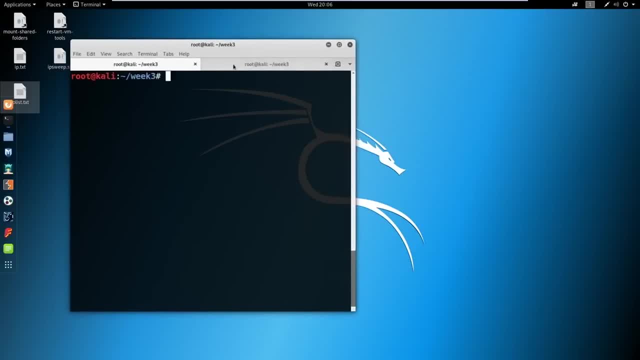 reason. So I've gone ahead and just opened two tabs here. I've made a folder called week three And we're going to do just a little bit of more advanced Python- not really super advanced Python- And then we're going to work on building our shitty port scanner. 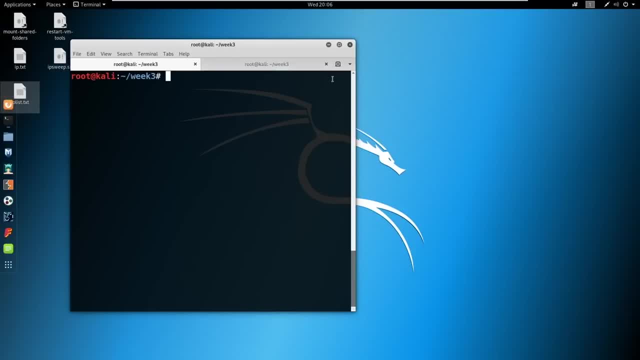 So once we do that, we'll do our giveaway, Q&A, and we should be good to go. Okay, let me get my notes up really quick here. All right, so we're going to open gedit And we're just going to call this. well, this is Python 102.. We'll just call this 102.py. 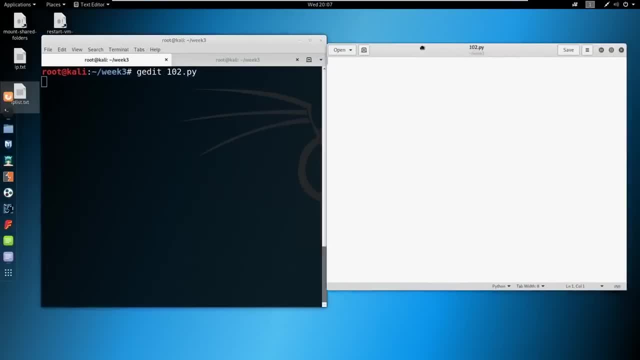 And I know you guys like this kind of side by side, like this, So let me do that for you. Okay, and let's declare at the top that this is Python 102.py. This is going to be Python 3.. And the first thing we're going to be talking about is importing, specifically importing modules. 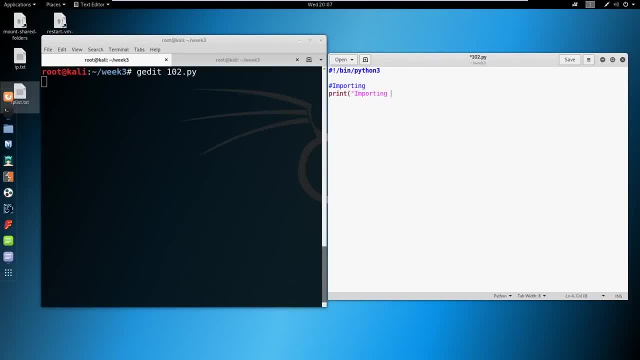 Like last time, I just want to print something here, So importing is important. That is a shitty pun, by the way. Okay, so what we're going to do is I'm going to show you a couple of basic modules that we're going to be talking about. 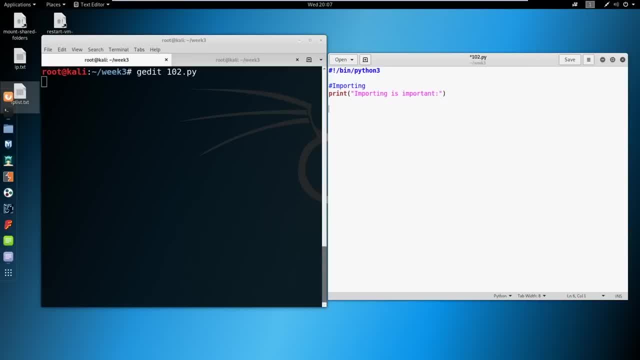 And then we're going to do a couple of basic modules that we're going to be talking about. Typically, when we import, we import at the top. So if we are going to import something, we would probably put it up here. But for the proof of concept, just keeping our notes organized, I'm just going to put it down below. 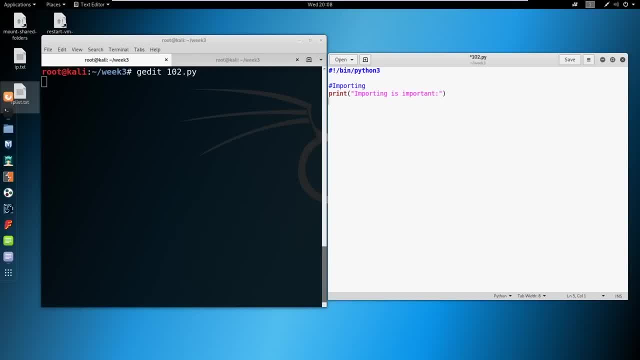 You'll see what importing looks like later when we actually build out our port scanner. Okay, so let's import sys, So we can import sys and we can just say: this is system functions and parameters. So if you think about like a system argument, which we'll see here when we build out our script, 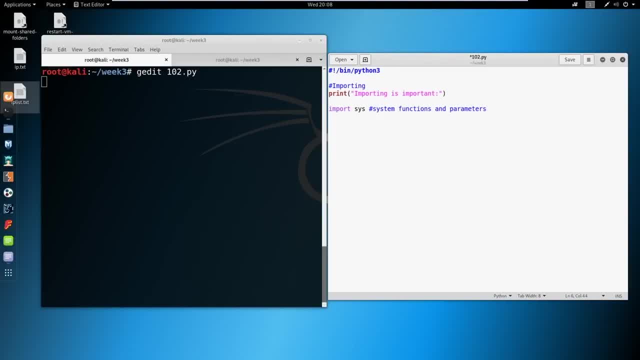 when we take an argument from a script, sys is needed for that To exit out, we need sys as well. So you'll see that in a little bit. So also from modules we can import a specific part of a module. So we can say: from this module, so from date time we'll just import. 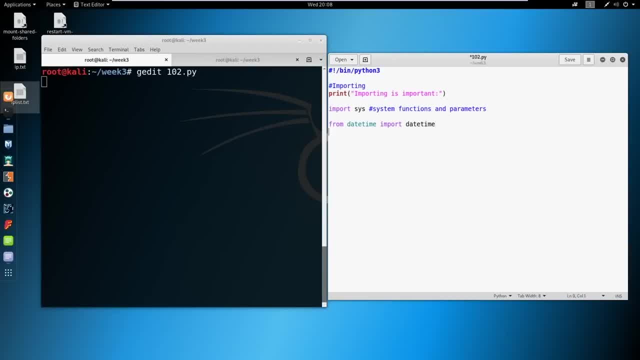 Date time. Thanks, Lee, I'm glad you like my pun Okay. and then we can say print date time dot now. And we can save it If we come over to here and just say Python 3, 102 dot pi. 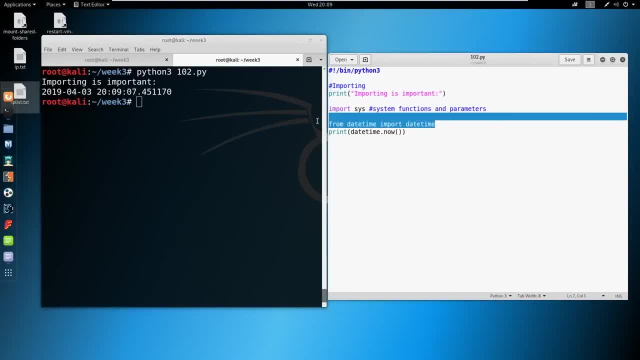 you can see that it prints the date and the time. So if I copy this and I delete it, save it And rerun it, you can see that date time is not defined. We actually define that in the module that we import. 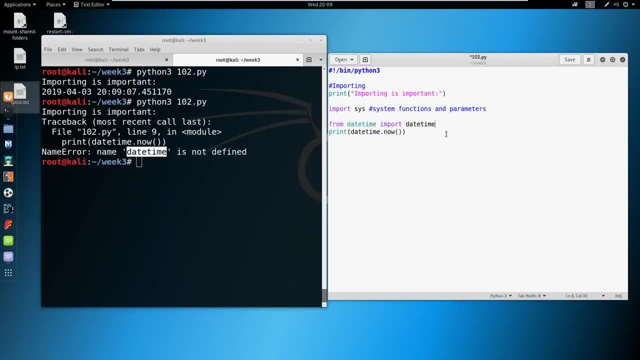 So this is why importing is important. Okay, and also we can do an alias with this. So let's say we wanted to import date time. I'll just show you again And then we'll import it as something else We could say as dt. 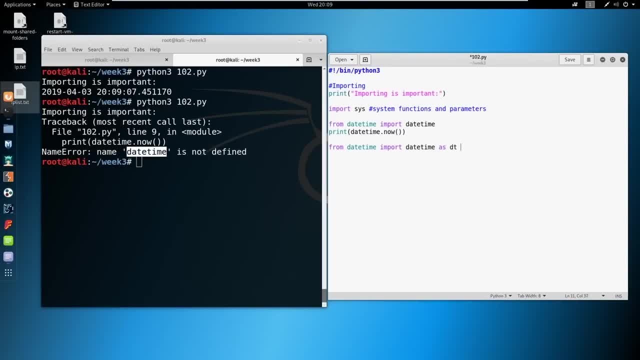 Say: we don't want to call it date time, We just want to call it as dt. We can call this importing with an alias And instead we can just say print dt, dot now, And we'll get the same results. So there you go. 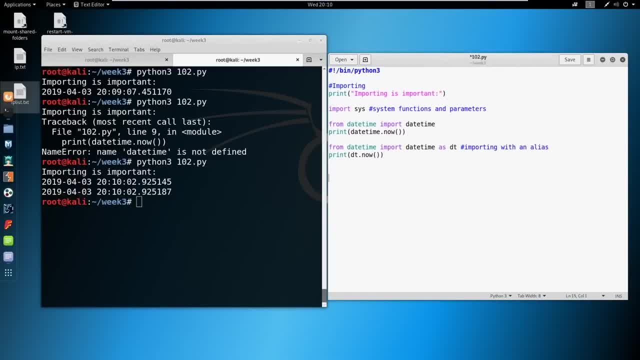 And because you guys complained last time about my copy and paste of a new line, we will define a function called new line And we will print a new line every time. So now we'll call new line, Let that print, And we're going to move into advanced strings. 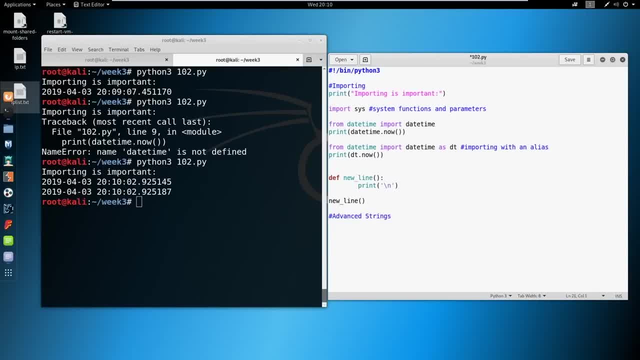 If I go too fast, let me know. I'm just trying to save time, since we are in a little bit of a crunch tonight and I want to spend more time on actually building out the application itself. So let's print out here. we'll just call this advanced strings. 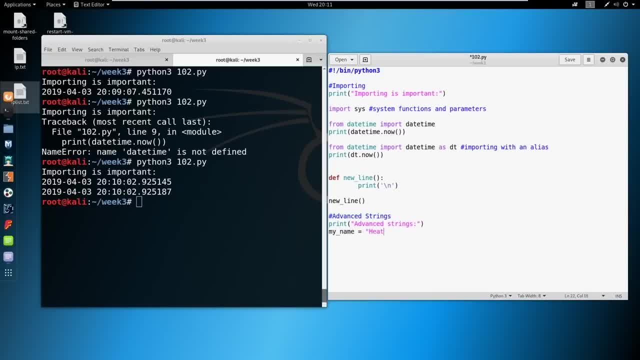 And let's create a string with your name. So my name is Heath. So, similar to what we were doing before with lists, we can actually call out parts of a string here. So remember last week if I said to you I want to grab the first initial of my name. 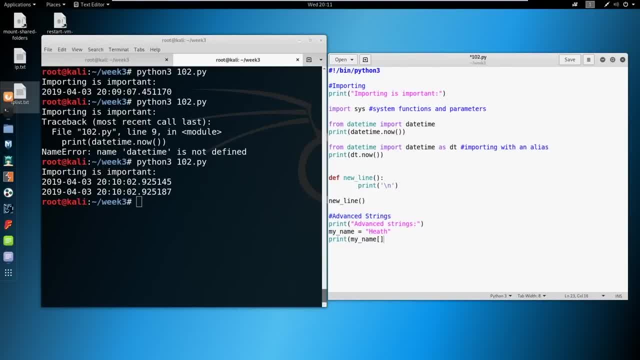 how would we grab the first initial of this name? Okay, Any guesses What number goes here? Zero, Okay, good, good. Now what if I wanted to grab the last initial of my name, or last letter? I guess not initial. 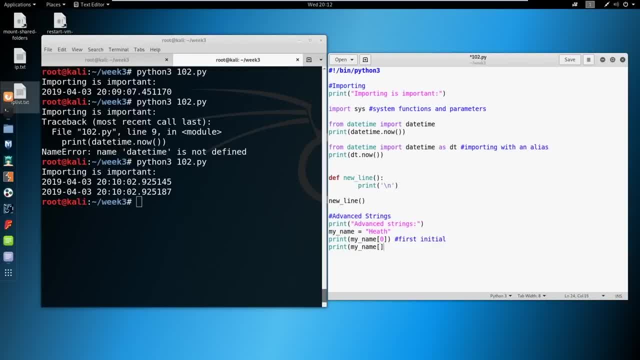 How do we grab the last one? Okay, We could use length, We could use four. Ah, look at you guys. negative one, Let's check it and make sure- Yep H, and then you see the little h here. So remember, negative one takes the last letter or last object. 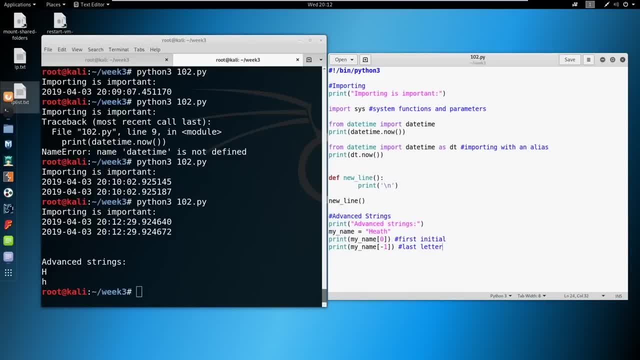 So remember, we started zero, we go all the way through And then we can have negative one. Let's try this again, but let's try it with a sentence. So let's say sentence, we'll just say this is a sentence. 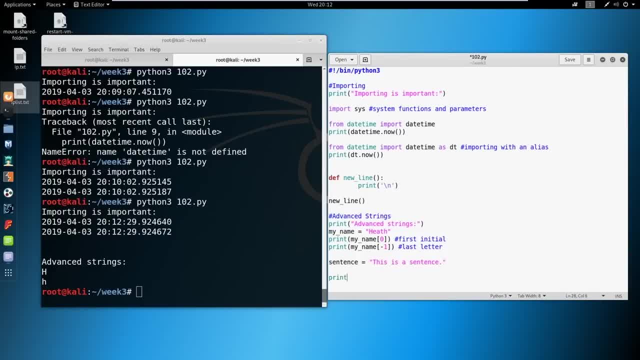 Okay, now I want to print the sentence. And what do I put in here, if I want to select the first word? I want to capture this. Okay, What are we going to put in there? I'm testing your knowledge from last time. 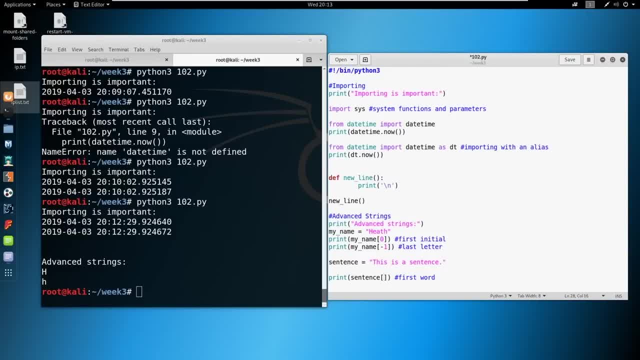 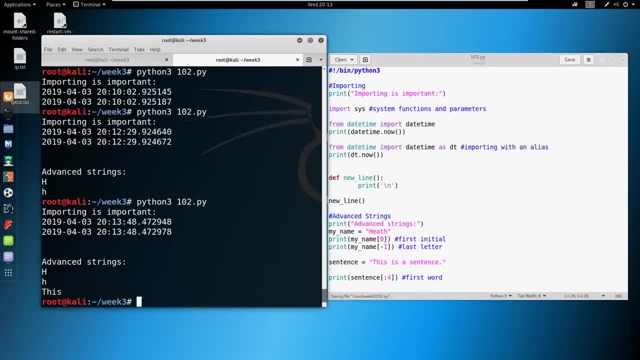 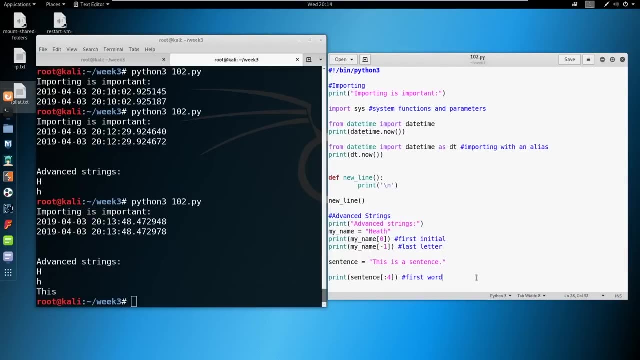 If we do it like this, we should be able to capture the word this: Okay. so, similarly, what if I wanted to capture the word sentence? Now, there's a couple of ways we can do this. I'm looking for some negatives. 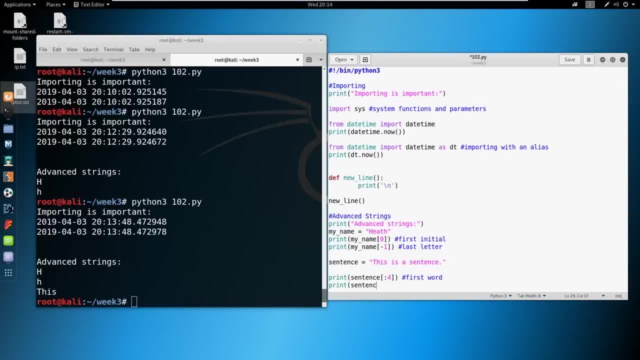 That's my hint. We're keeping it simple, Very, very simple. Got to vote for negative one. got to vote for negative eight. got to vote for negative nine. Okay, negative nine is the correct answer. Now what if I don't want that period? 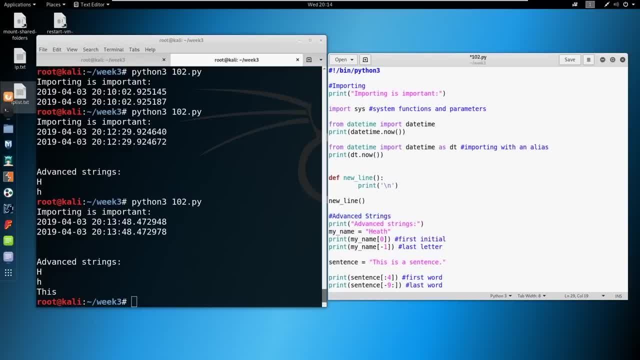 Okay, We could strip off the period. but what's an easier way to just get rid of the period? in this sense? We know the word, we know the amount of characters. Just for basic thinking process here, We could remove it from the string. that is absolutely correct. 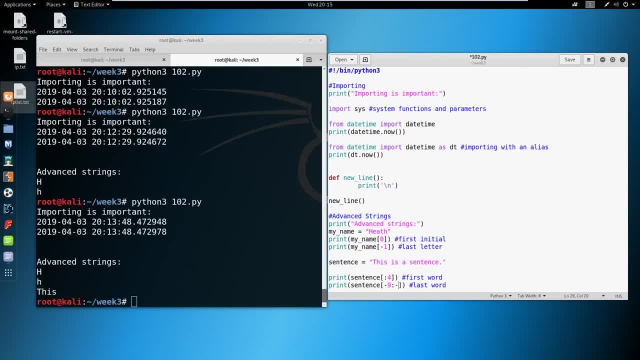 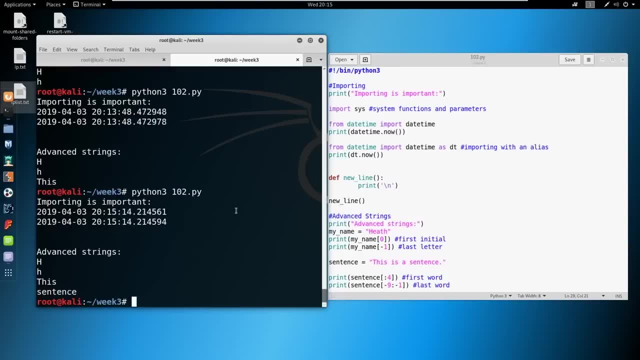 What about a negative one? Yeah, there you go. So we can also write it like this, So we can go backwards with the negatives, And now you see, we pull out the word sentence. So just food for thought that we don't have to go from the positives. 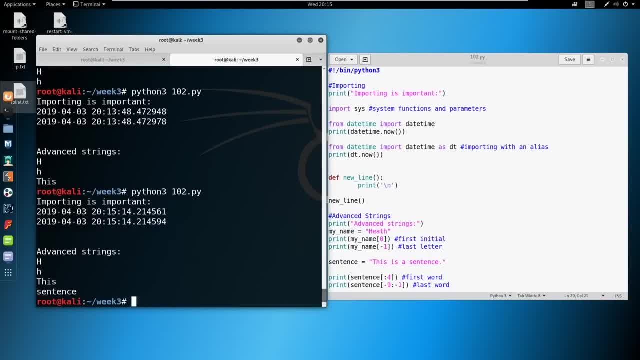 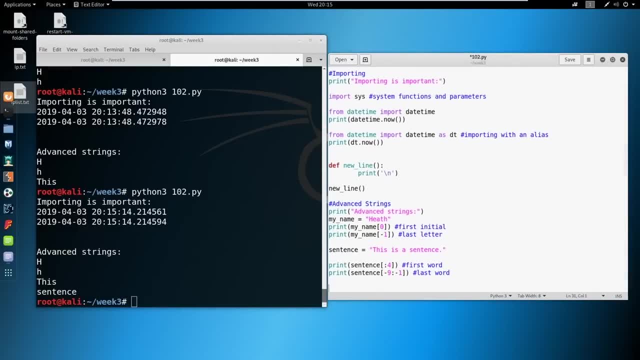 we can also take it backwards with the negative. Okay, so a couple more tricks with strings. Do you want to see what negative zero looks like? We can check what negative zero looks like. You get T because there is no negative zero. 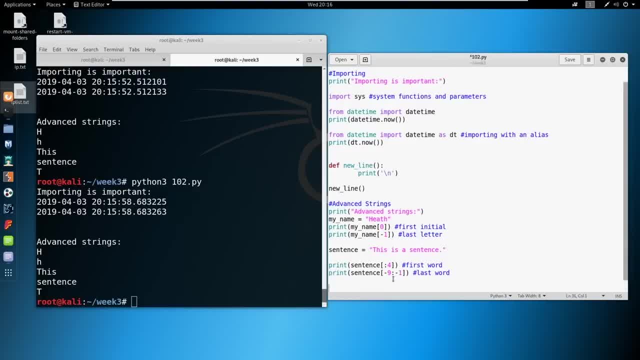 It's just zero. All right, let's talk about using split. So let's say that we wanted to split sentence into every word that there is in sentence. So there's four words, right? Well, we can just say: print sentence dot split. 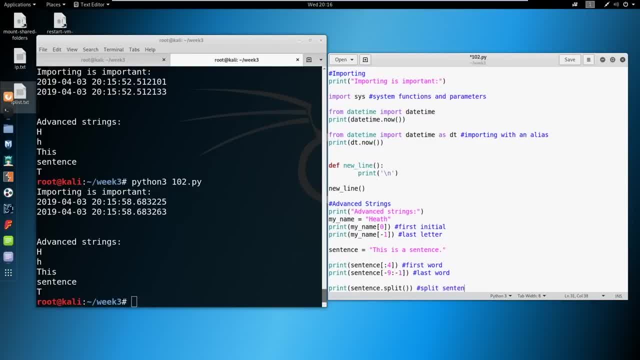 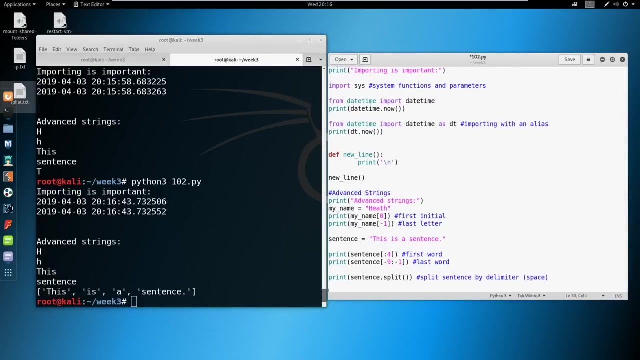 And automatically split the sentence by delimiter, Which is going to be a space, Right? so we've got the space by default. So it'll say: this is a sentence. Now we could also do this, for say example, here we could say: sentence split equals sentence dot split. 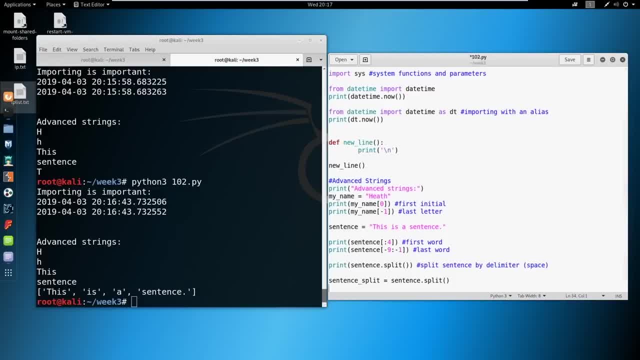 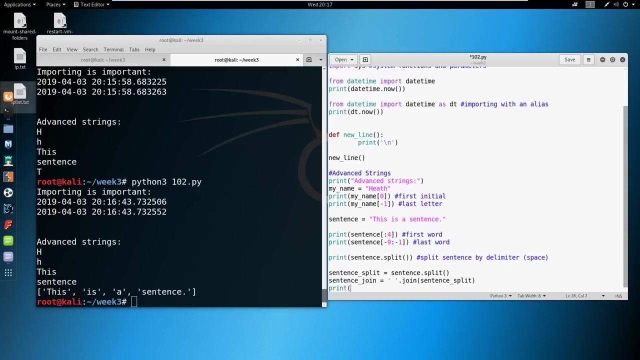 Right now we split it out. What if we want to do join everything back together? Well, we could say sentence join, And we can also provide a delimiter here of a space like this. We'll say join, sentence split. And if we were to print sentence join, it should look just like the sentence that we had. 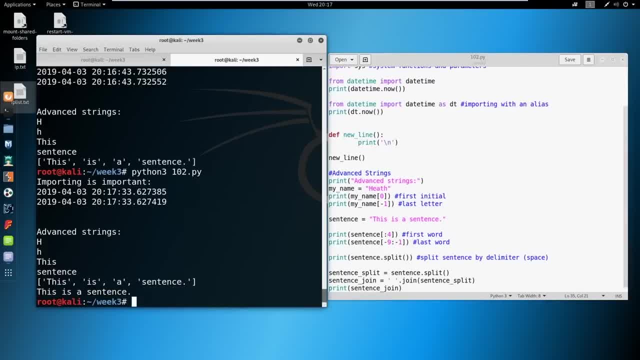 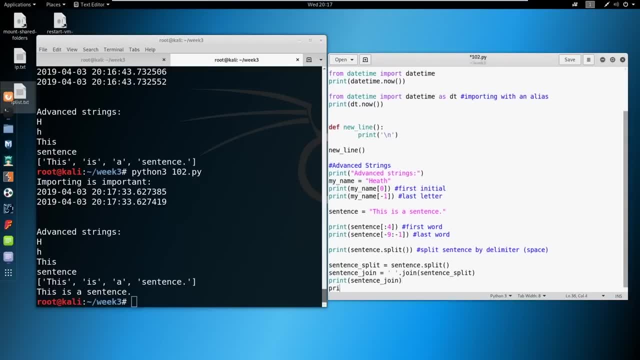 Even though we stripped it down. now, you see, it comes back to this as a sentence. But for a other proof of concept, we could print something like print: We can give it a new line for every one. Just put a new line and say join. 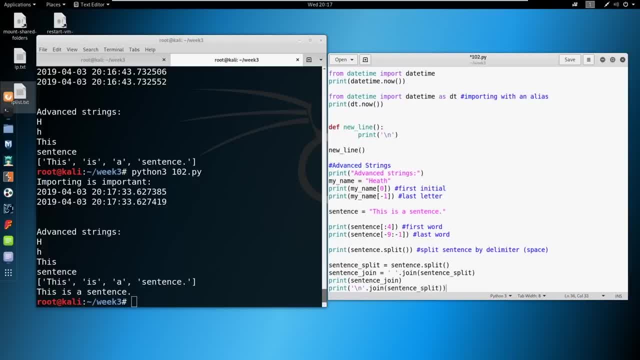 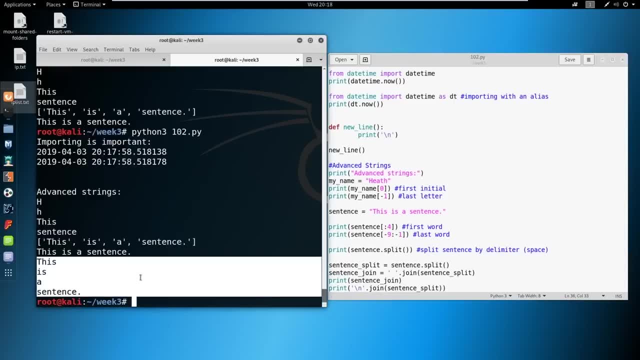 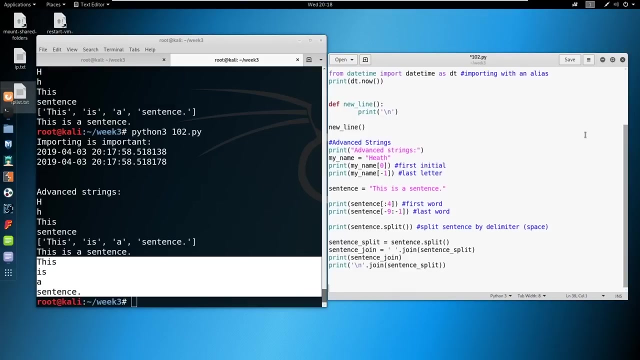 And say sentence split, like this. We won't put it into a variable. If we save that, then you see, this is a sentence, So we can break these down and put them back together and structure them how we want. Okay, so something that I didn't show you guys last week is escaping. 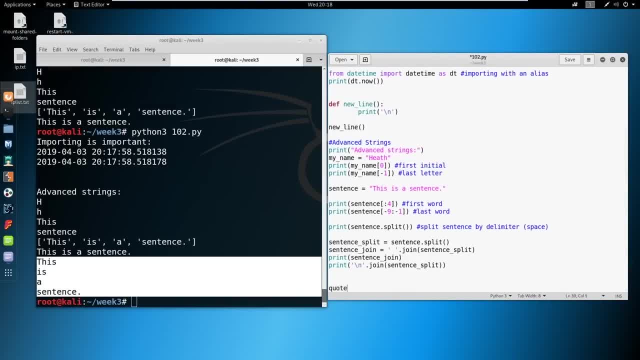 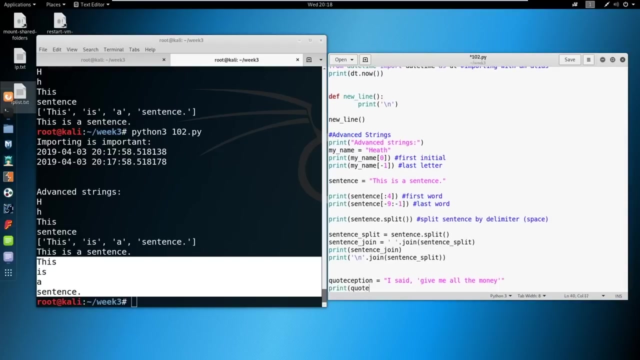 So let's talk about quotes inside of quotes. We'll call this quote-ception Because I like that. So we could say: I said: give me all the money, I like money, And then we just print Quote-ception. 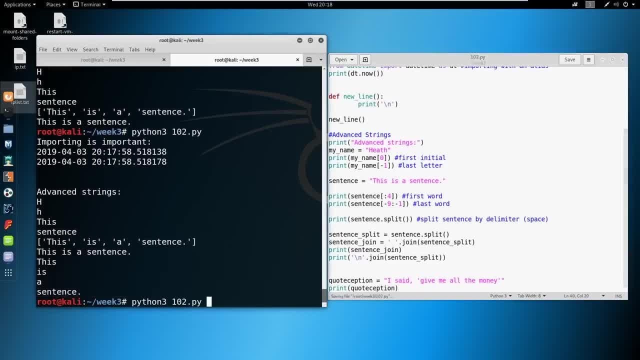 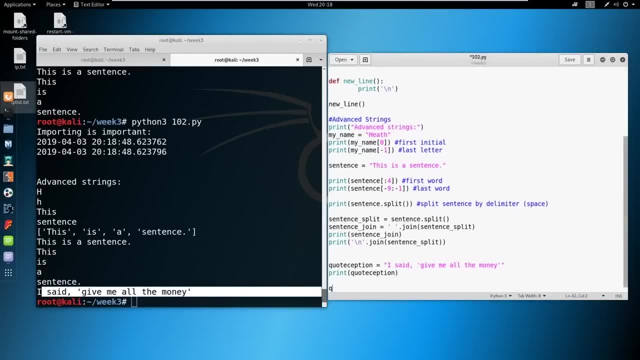 Right, And how is it going to come out? Comes out alright. What if we did quote-ception now And we said: I said, give me all the money You could see? this is kind of an IDE. It's not a real IDE that we're using. 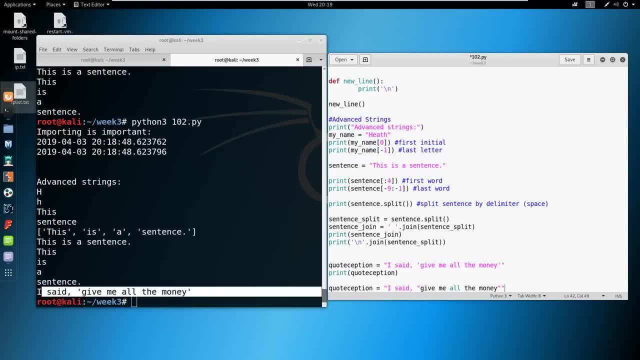 But it's giving us a hint. It's giving us a hint here that something's off, Right? We're seeing that it's not all pink like it should be. It's actually taking this And if you see, here we've actually ended our string. 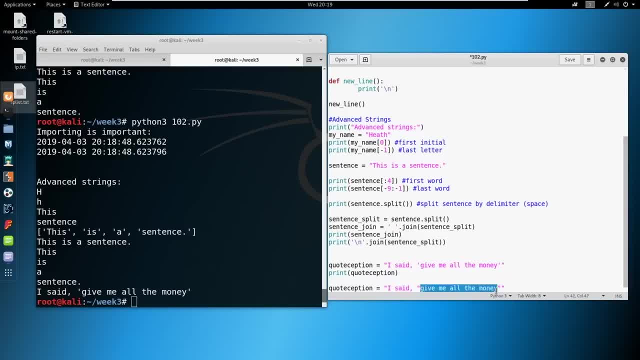 and begun a new string And everything in the middle is just kind of wonky. It is definitely invalid syntax. So how can we make this valid? Well, we can do this Triple quote that shit. We could triple quote that shit. 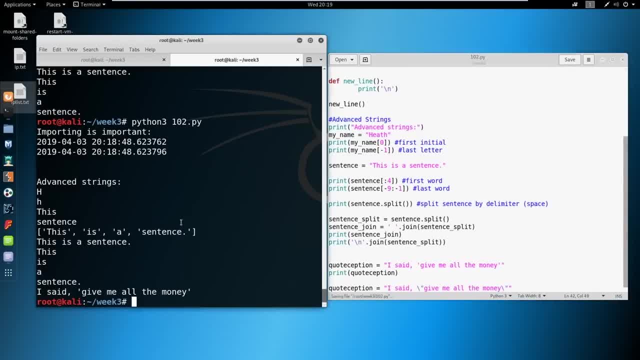 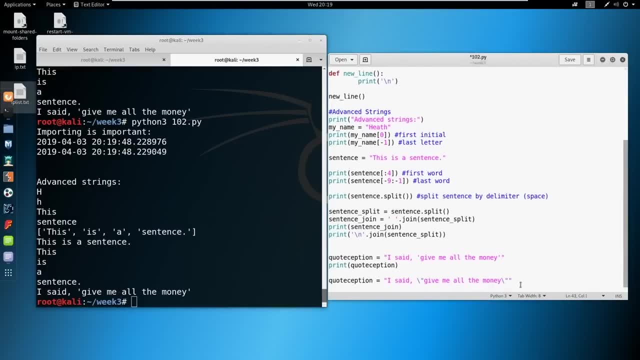 Could also do this. right, Put some escaping in there. Except I didn't print it, So you wouldn't know if I was correct or not. I could be lying to you. And there you go. I said: give me all the money. 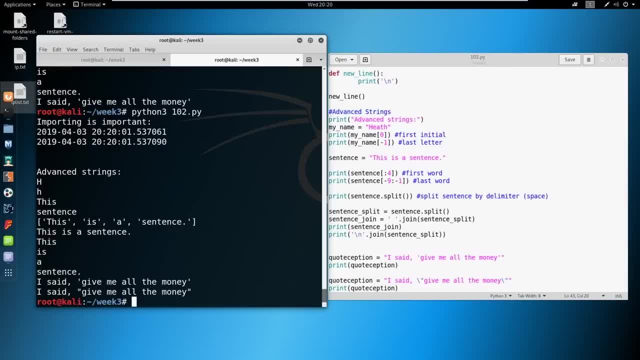 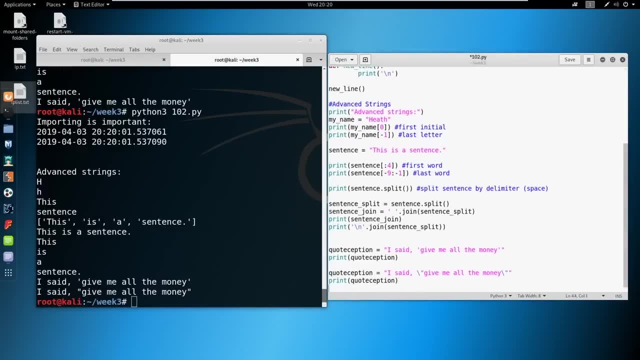 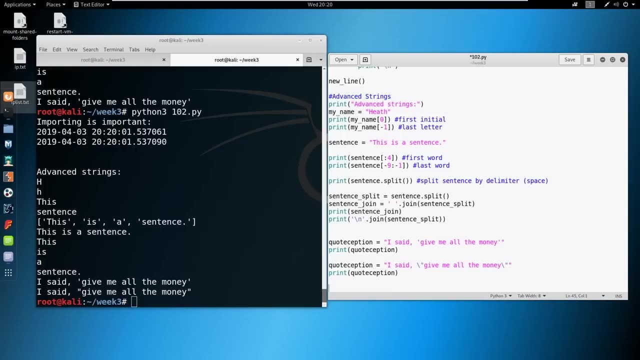 So that was something I probably should have shown you in more of basic strings, But it fell into advanced strings. You don't know that, Jeff, I might lie. All right, So now let's talk about a couple more things, and then we're going to dive into dictionaries. 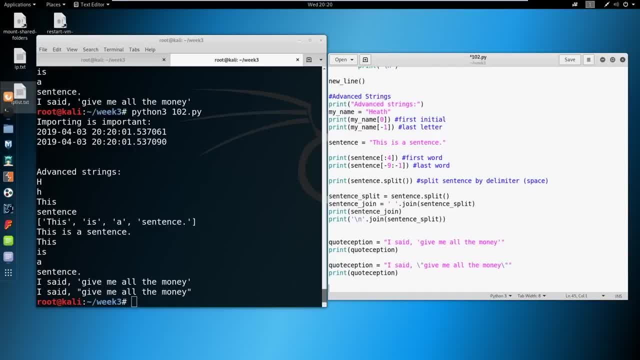 You don't have any money. I don't know about you, man. Okay, What if I said something like this: Print A in Apple. What might this return? What does this turn into? Do we see A in Apple? It is Boolean. 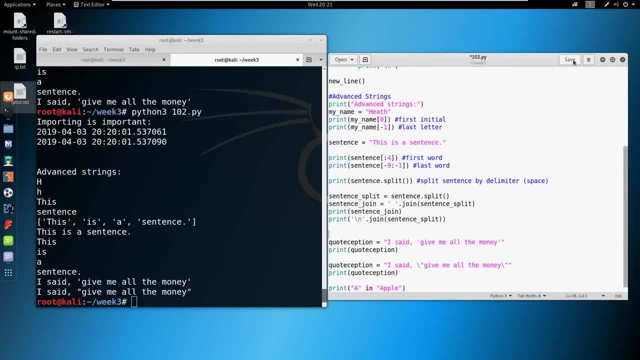 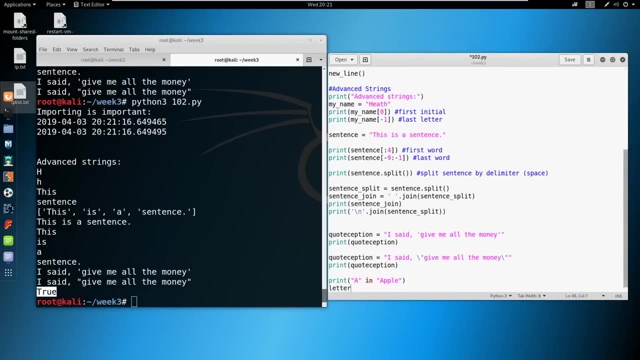 It is absolutely Boolean. So this is true. Right, If we were to print this, it returns true. Okay, Let's get a little more complex and change our logic a little bit into how we think. Let's define a letter. Call it A: 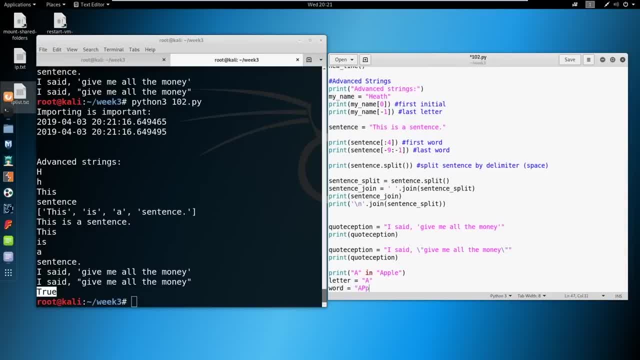 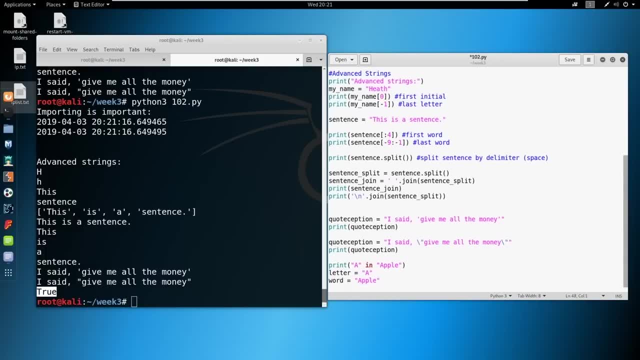 And let's define a word, Call it Apple. Now let's do a couple things. Let's say print letter in word. Okay, So that should still return. true, right, But what about? what about this? Is it Scott? 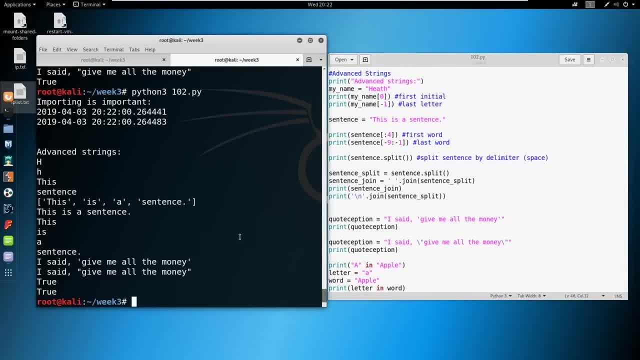 Pick one, Okay, So I'm gonna set that down as our new code to start using this new code. So we're gonna make that look like, not edit, So the chat's not up for those watching this video later. The question asked is: will you put all this code? 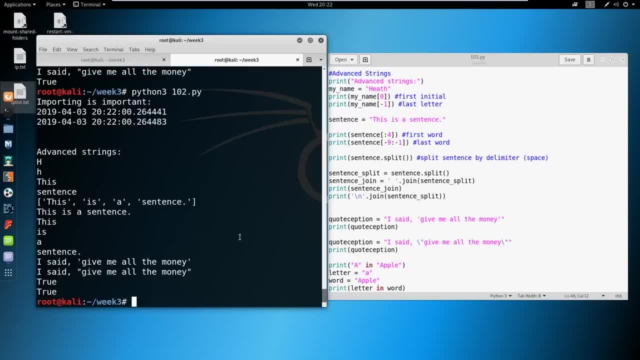 on a paste bin. when you're done, I will put it into a note on the Discord server. If you're not in the Discord server, do get in there. There's a zero to hero channel and I'll put all that When this whole course is done. 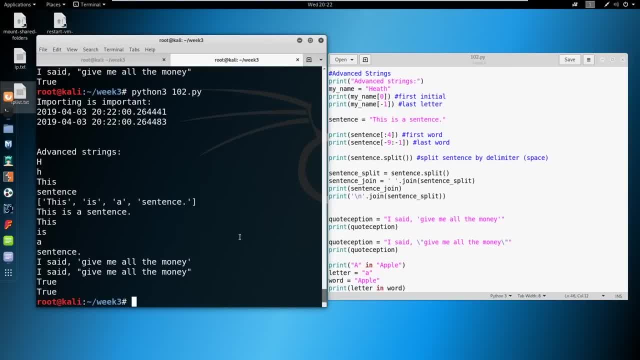 I will make a collection and put it somewhere place. I'm just one person and I am very slow at what I do, So okay, So if we submit this now with the lowercase a in Apple and we print it, 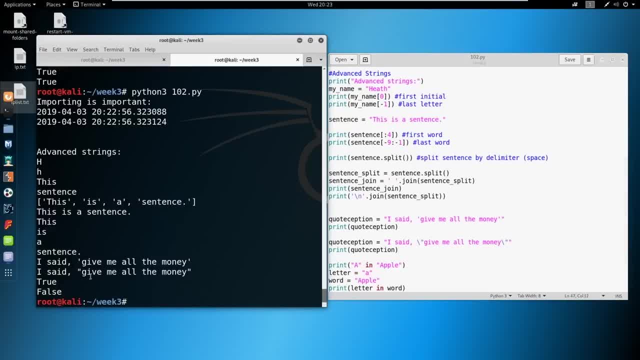 you see now that it says it is false because we have a lowercase a. even though this letter is in here, it's not matching syntax, Okay, well, how can we fix this? Any ideas? What would be the thought process behind fixing something like this? 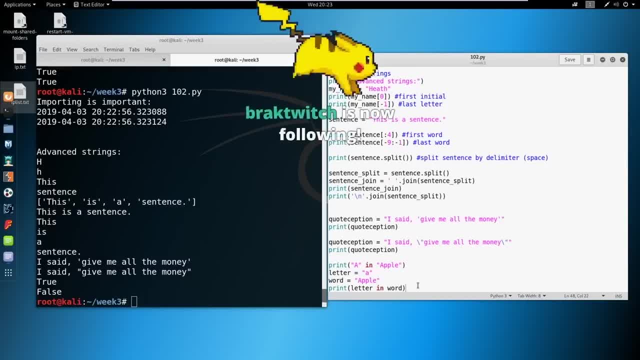 Logically, you don't have to know the syntax or anything. Somebody have an idea? A or a, We could do that. Upper would work, or lower would work, Very good. So what we're going to do is we're going to say letterlower like this: You could also use upper. 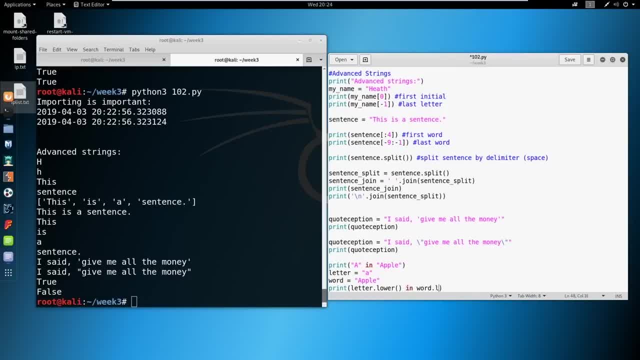 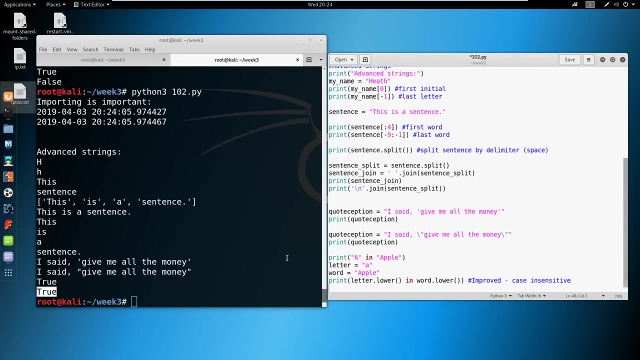 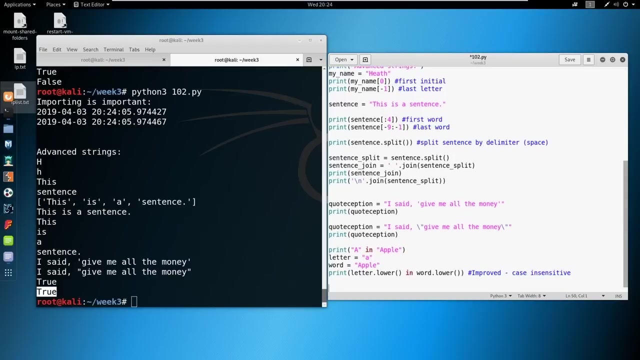 in wordlower and let's try it now. And now it returns back to true. So it is case insensitive, correct? Everybody is correct. We'll just call this improved case insensitive. Okay, One last one. So this is just. 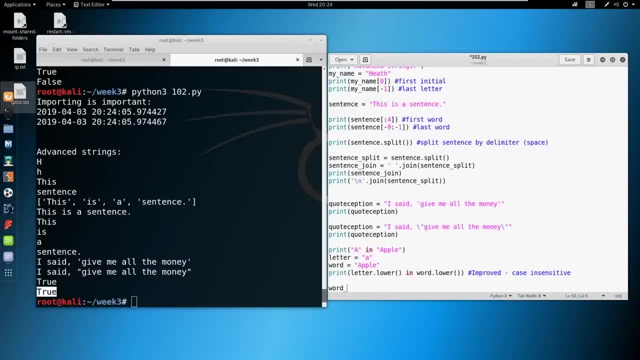 Okay, a demonstration of something we saw last time. we saw the use of not, but we didn't use it. we didn't use it a lot, right? so i want to show you just a quick printout you can copy along real quick. let me type this up. 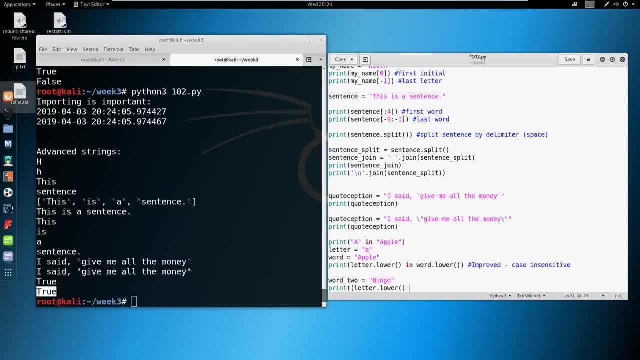 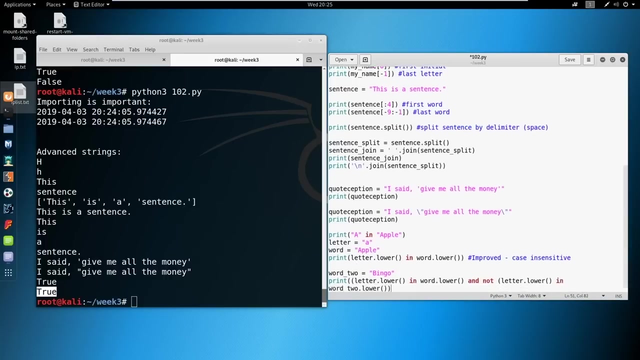 basically i want to say: okay, is letter in word dot lower and also not letter dot lower in word two dot lower. miss syntax here. just make sure you have the triple. if i type this right, it should return true. okay, so remember, this condition is true and this condition is false, but it's not false. 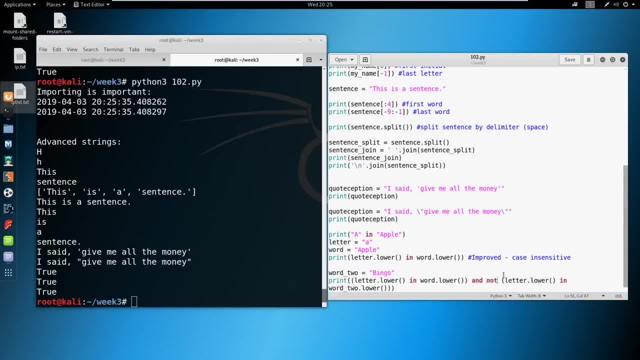 so true and not false is true and true. thus, we return true now if this is, or we would return true regardless if it was true or false. on the second condition, just want to give you one more look at a boolean and another one that is using, not because we did not cover it as well as i'd like to last week. 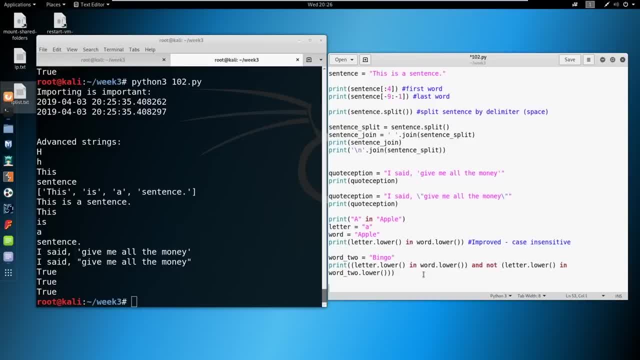 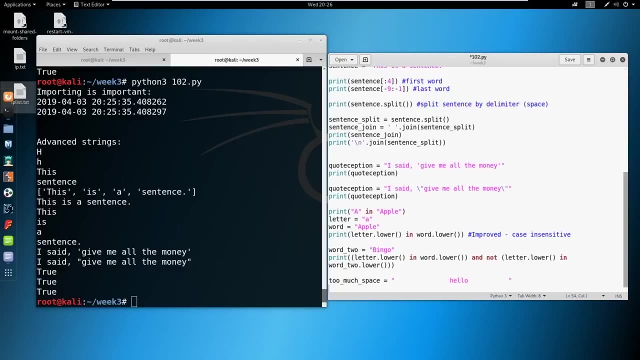 okay, a couple more things. so let's define a variable called too much space. let's just say however much space you want to put in there. we'll just say, hello, now if we wanted to get rid of all the space that's here. we'll just say: print too much space. 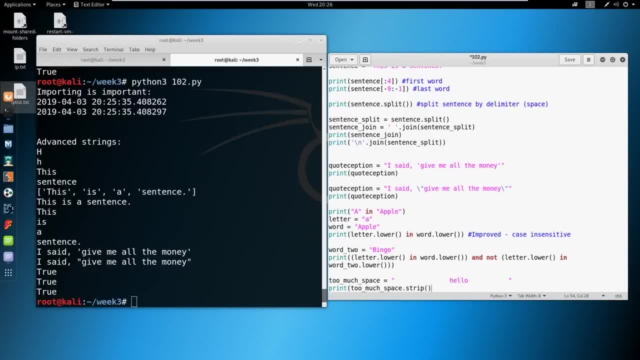 dot strip and the delimiter that we are stripping by by default is a space, so it should remove everything that we have in here. you see there's no spaces on the first bar around it now, So you can strip whatever you put into here, but by default it is going to be a. 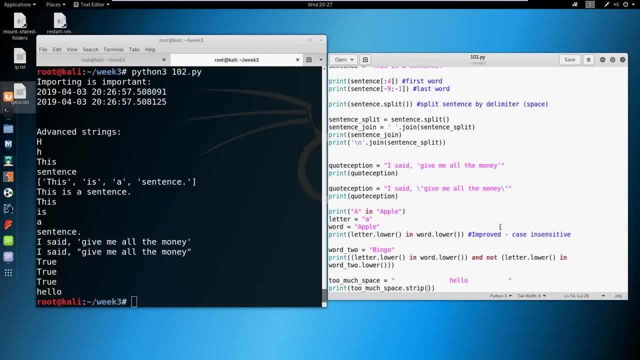 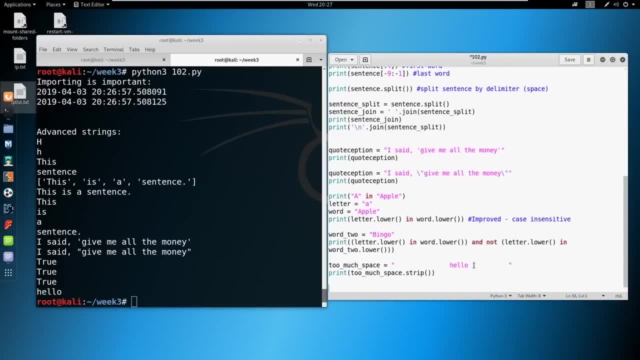 space. Okay, so let's look at some other examples as well. Let's do full name. So my name is Heath Adams, but let's say I missed the letter when I typed it in and I need to fix that. Well. 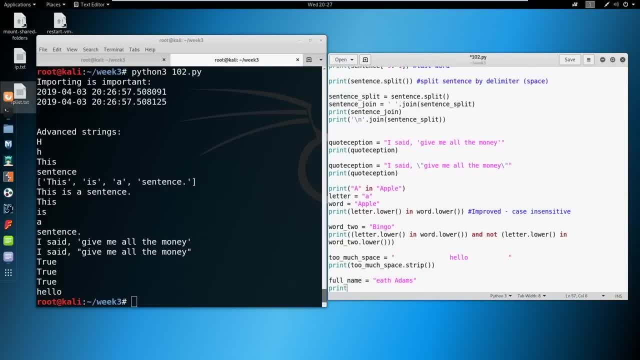 strings themselves are immutable, right? We can't change a string, So I can't just add an h into here. We can make a new string or a new variable, but I can't improve or add upon what I already have. However, we can print out: 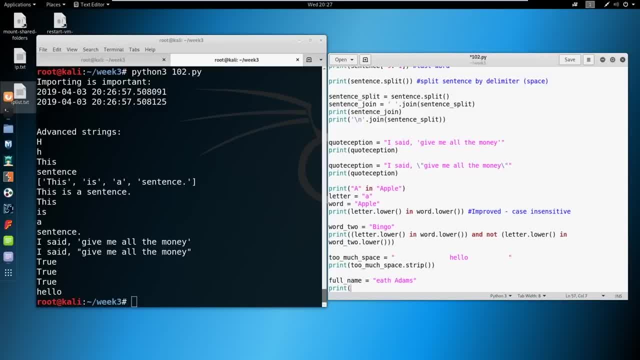 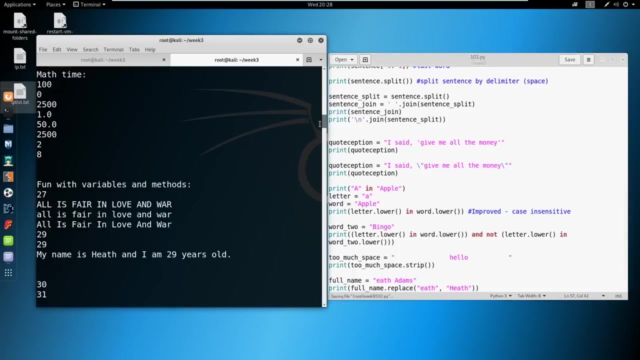 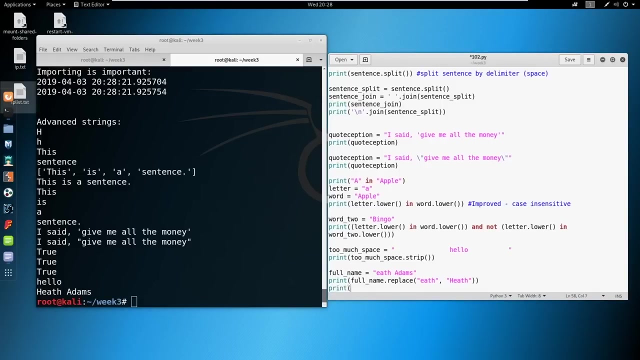 So let's say full name. You guys are getting ahead of me with the placeholders. We could say replace, and we say eth and instead say Heath and then save and print that and now you see, it says Heath Adams. Another useful trick is: let's say we want to find the point in characters or position where a letter 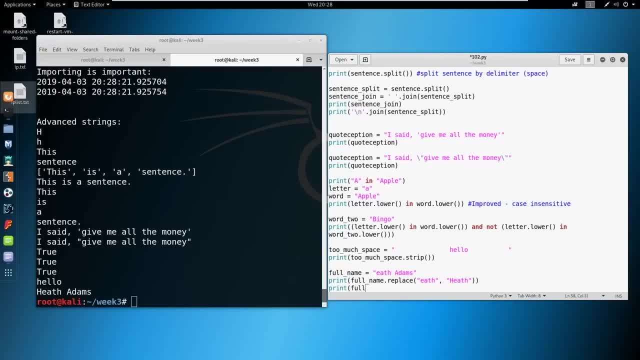 occurs or a string occurs. So let's say full name. We can use find. Let's say: I want to find where my last name occurs in this string, right, Okay? So let's say find occurs at position five. So all it's going to show you is where that a lines up. 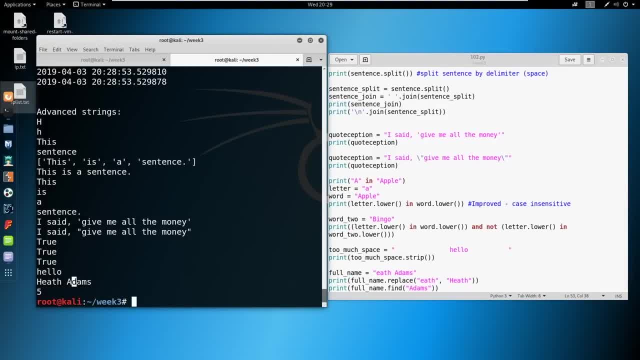 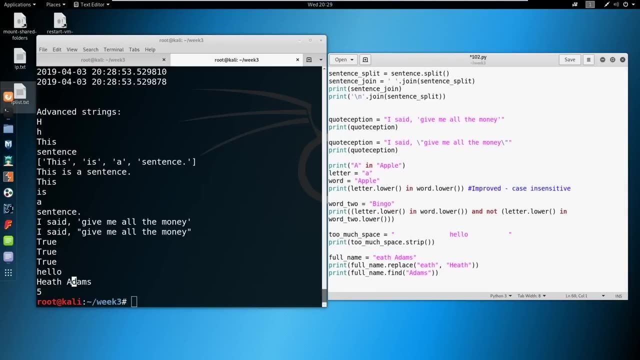 with that a and give you that return area, So could be useful in the future. Now, since you guys got ahead of me, let's move into placeholders, and these are going to become useful. We're about to use these when we write our script So we can define a variable. Let's define a variable of a. 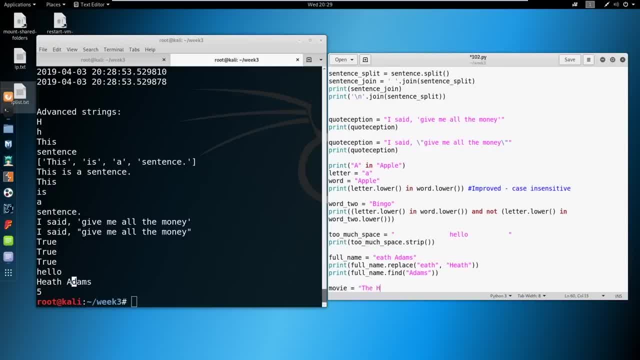 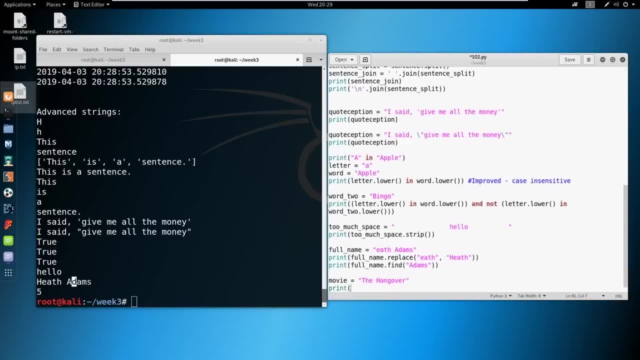 movie And we'll just call it the hangover. we use this last week And let's print out: my favorite movie is: and now, typically I would do something like space movie- right, We could do that, But what if we had? 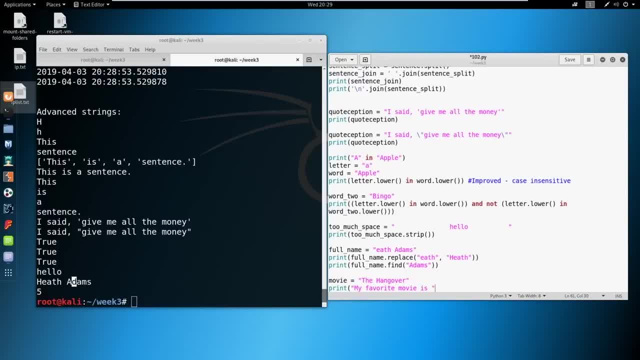 like you know, a long sentence and we didn't want to keep going and concatenating here. Well, we could use a placeholder, Something like this: I spelled favorite wrong, apparently. All right, My favorite movie is: And then we can add a period format movie And it'll fill in that placeholder. for us. My favorite movie is the. 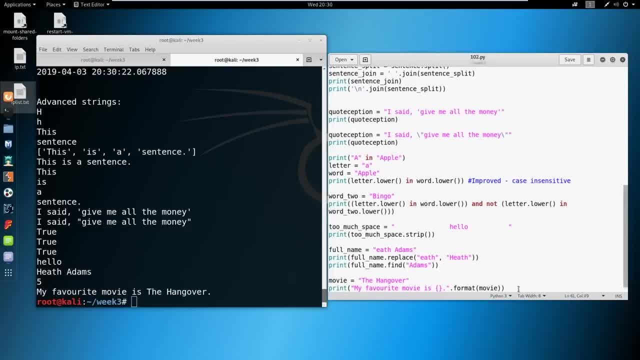 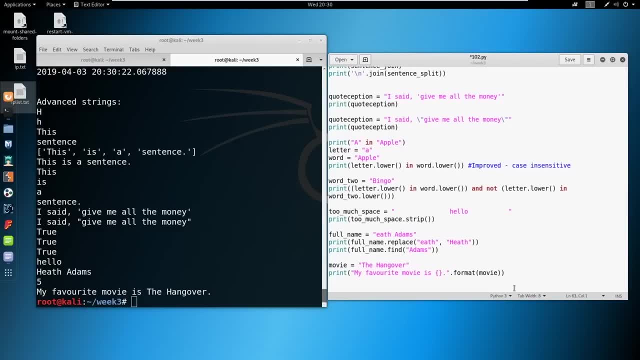 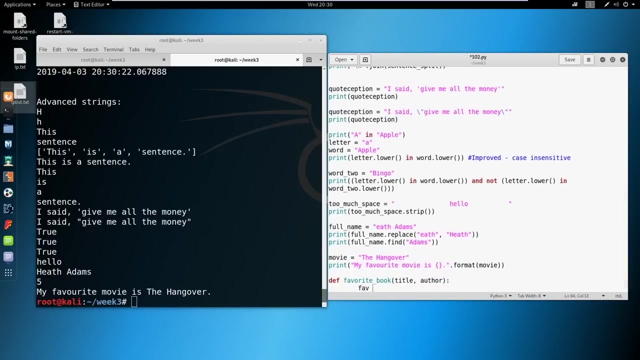 hangover. Okay, let's try something else. Let's try a couple parameters at once. Let's actually put it into a function. So let's define our favorite book, Let's get a title and an author Right. We'll define a variable called fave. 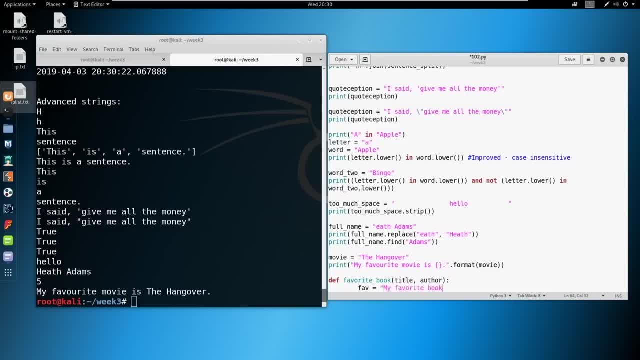 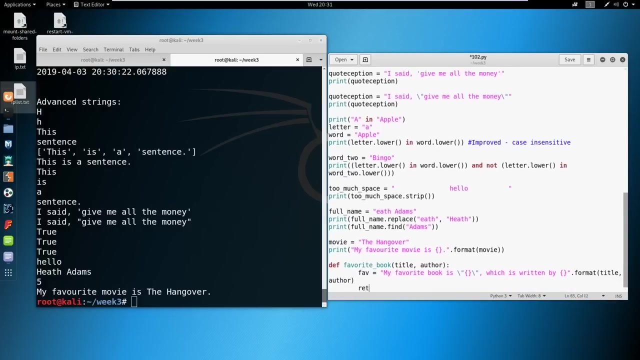 and we'll say something like this: my favorite book, we're back to the US spelling is: and remember we're escaping here, so I'm adding quotations- which is written by, and now we can say format: title, author, return, fave. 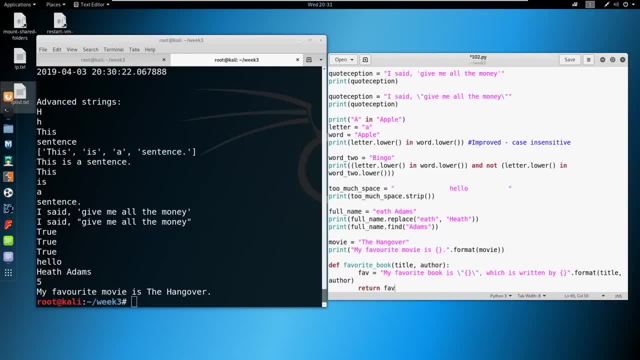 So you can use %s as well, just different types of placeholders. Sorry, if the string is hanging, guys, I am not getting anything on my end that's showing dropped frames, so I don't know what's going on. If worse comes to worst, you can watch the VOD. the VOD will be clean. 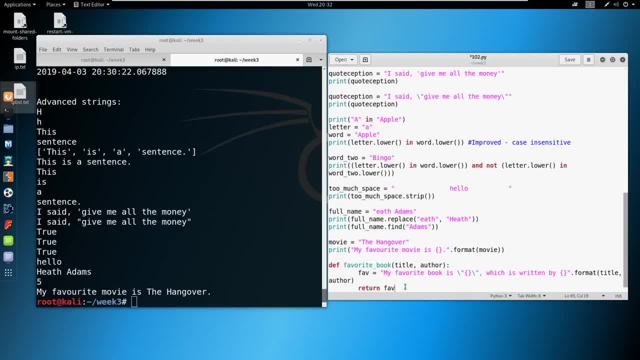 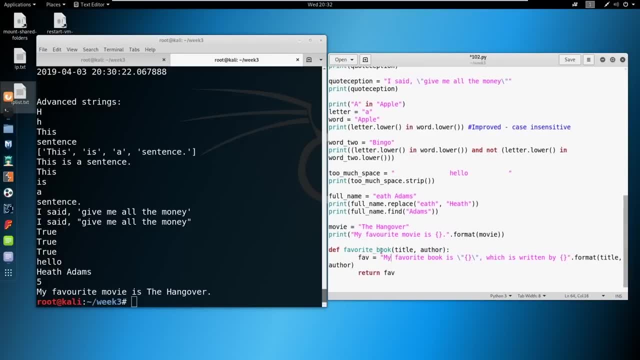 Okay, Okay. So let's look at this. So, if you see, the function takes title and author, we define a variable and we say: my favorite book is put a placeholder, which is written by: put a placeholder. let me add: 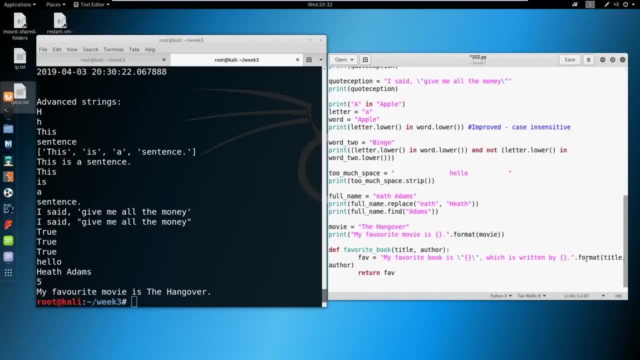 a period here, complete the sentence and then we format, we say title and author. Okay, so now we can print favorite book. if I could type, Let's say it's The Great Gatsby And favorite author is F Scott Fitzgerald who wrote it. 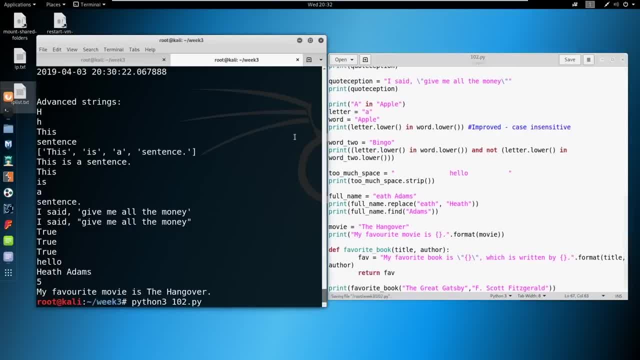 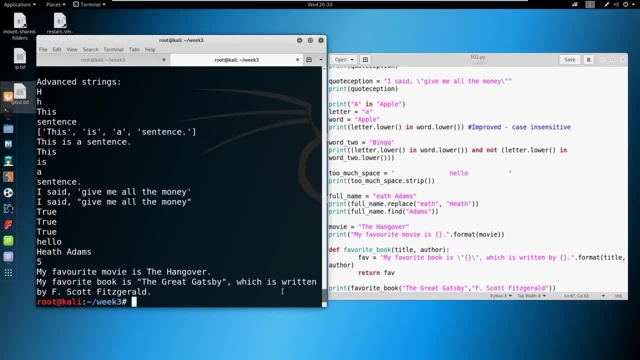 Now, when we print it out, it should read a sentence. My favorite book is The Great Gatsby, which is written by F Scott Fitzgerald. Great Gatsby- Okay, So incredibly useful to have placeholders. Okay, that is it for strings. 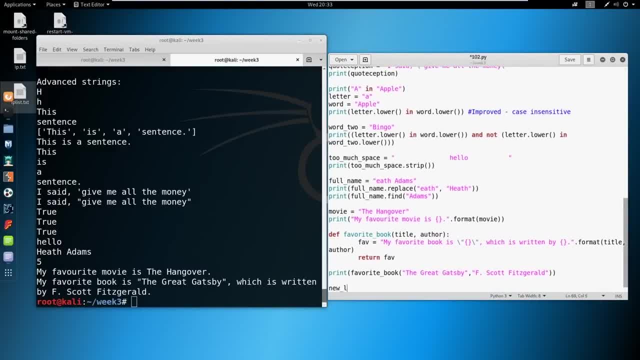 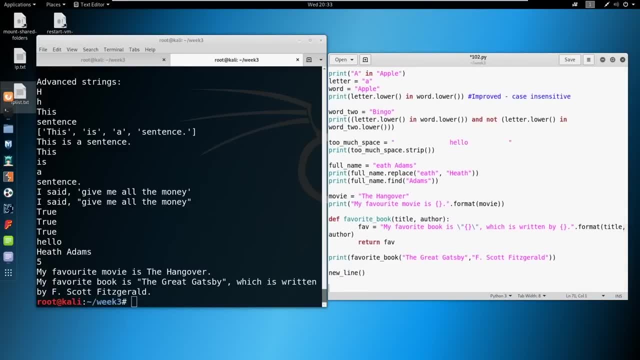 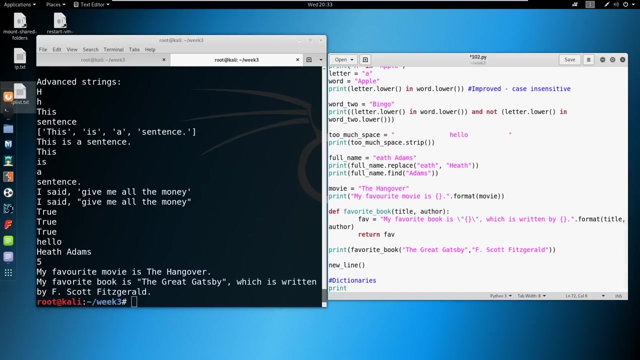 Strings and things. we are done, So we'll call our new line: We're gonna do dictionaries real quick and then we'll go ahead and write our cool little shitty port scanner. Okay, dictionaries and print Dictionaries are keys and values. 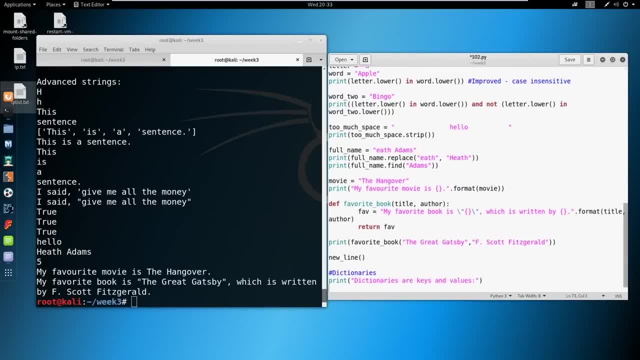 Okay, So in the past we have used lists- Right Lists looks like this. We've had tuples which are like this, And now we're gonna have dictionaries which are like this, So be able to identify the difference in bracket parentheses or whatever you call. 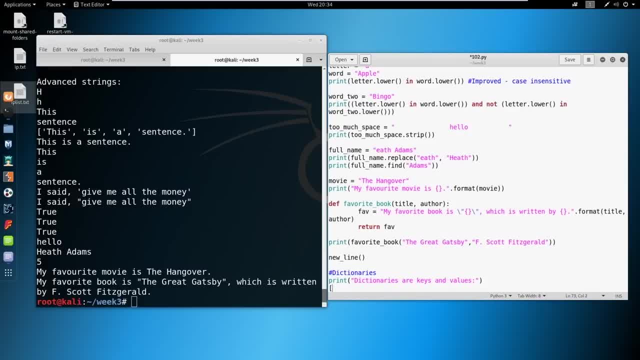 these squigglies? I don't know. Okay, Is that really how you spell dictionaries? Yeah, Okay, If so, that's awful. Okay, let's say we have drinks, right, And let's talk adult beverages. Say white Russians. 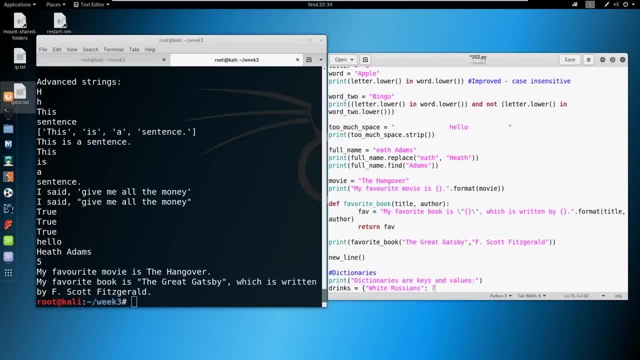 Let's say white Russians are $7.. Okay, So the white Russian itself is the key and $7. here is the value. Let's add some more in here. Let's add an old-fashioned: Call that $10.. Let's add a lemon drop: $8.. 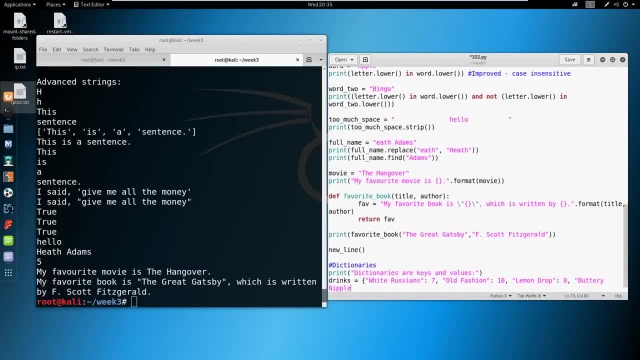 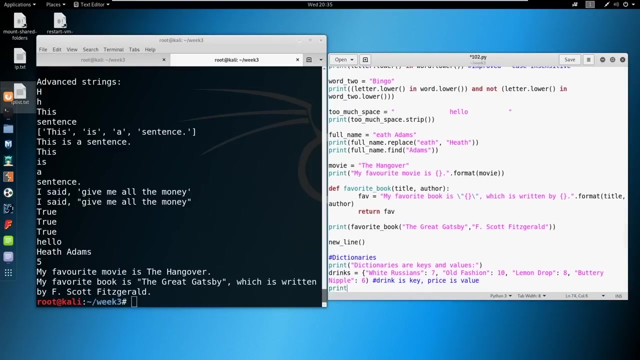 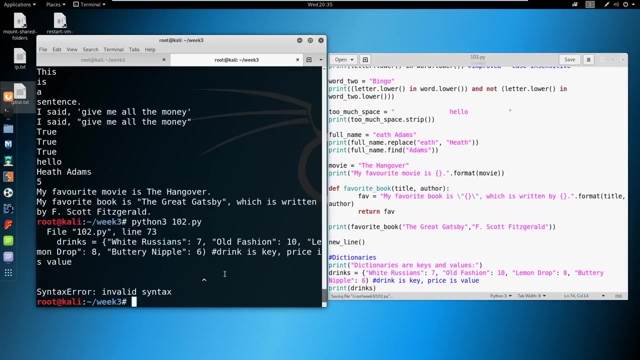 And, of course, everybody's favorite, the buttery nipple. We'll make that $6.. We'll say: drink is key, price is value. Okay, and let's print out drinks and see what it looks like. Syntax error. What did I do? 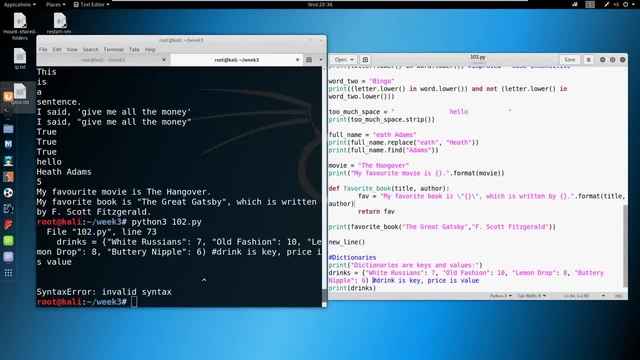 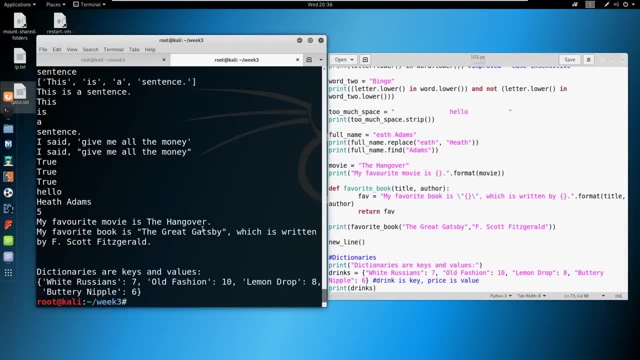 Aha, You guys, let me do this. Syntax is everything in Python? All right. so you see, it says white Russian: $7.. Old-fashioned: $10.. Lemon drop: $8.. Buttery nipples: $6.. Okay. 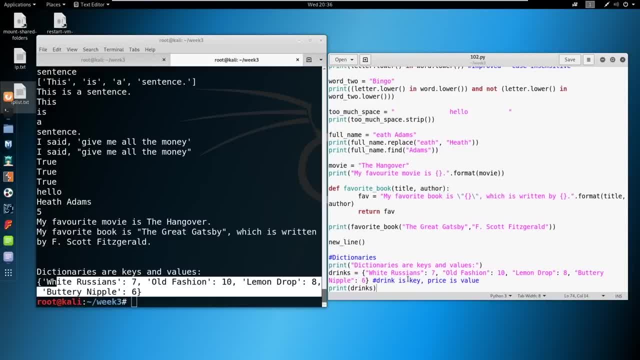 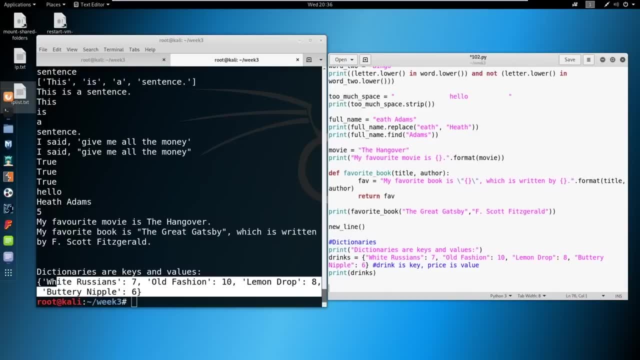 That's fine. Let's leave those alone for now. We'll come back to those in a little bit. We don't have to have a string. If we have a string and then a value, we can have a string and a string. 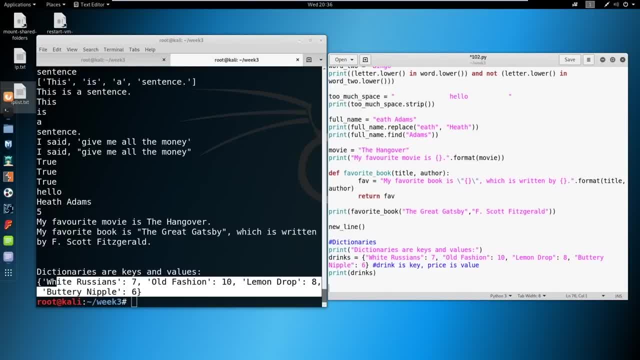 We can have a string and a list. Let's take another look at this. So let's say we've got employees and they work in different departments. Let's say finance has Bob Linda Tina. We'll say IT has Jean Louise Teddy. 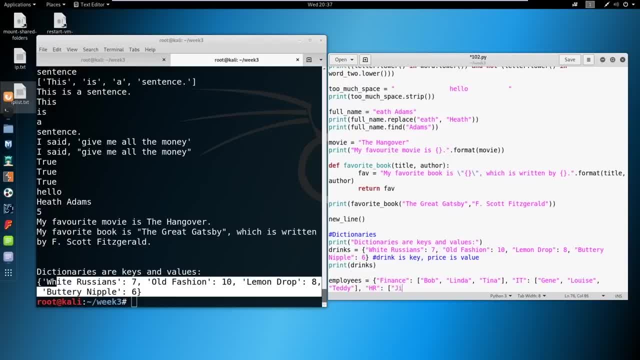 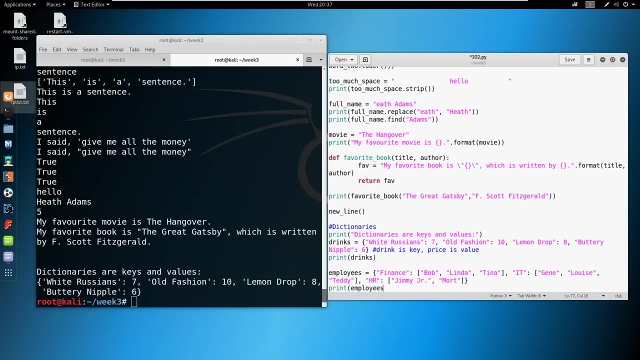 HR is going to have Jimmy Jr and Mort. Okay, All right, So we can just press print Okay And we'll close this off And save it. Let's just print it. make sure we did everything right Would be helpful if I printed it. 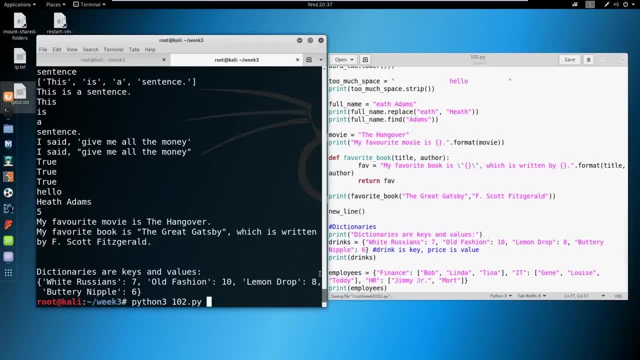 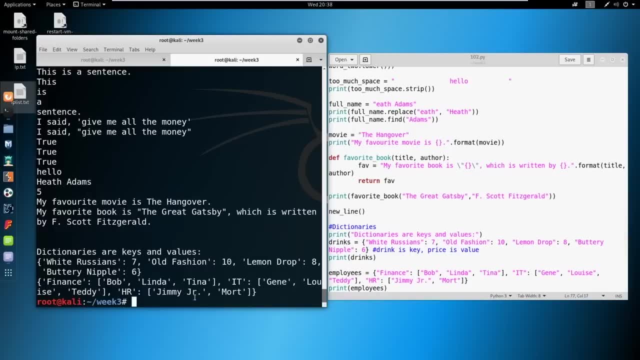 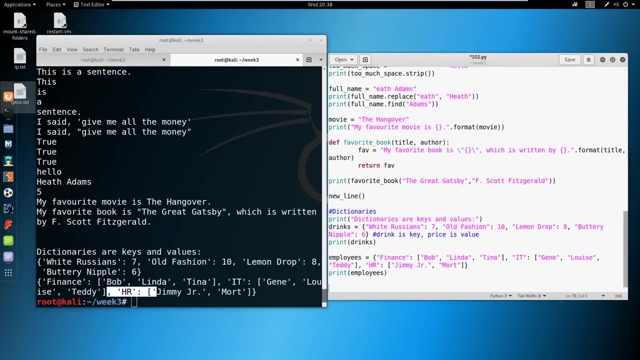 You hate Teddy? Teddy's- okay. I wouldn't say he's the worst, All right. So we've got finance, IT and HR. Let's say that we wanted to add something new. Let's say there's a legal department- right. 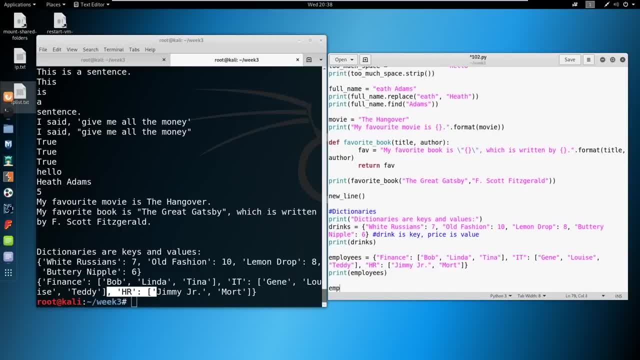 All right, well, we can just go ahead and say employees and there's something like this. We could say legal And let's add: let's say Mr Frond is in charge of the legal department, And all we're doing is we're adding a new key value pair. 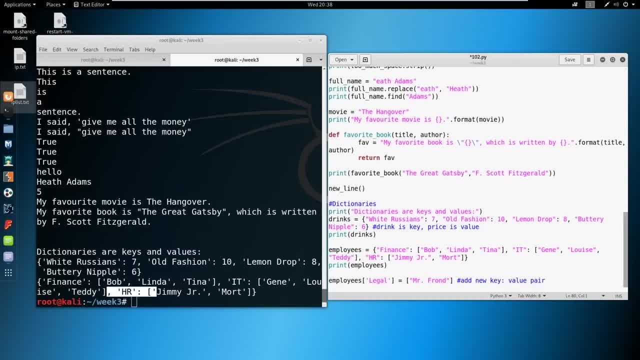 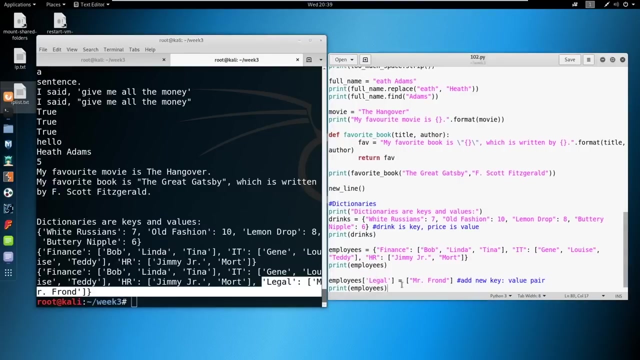 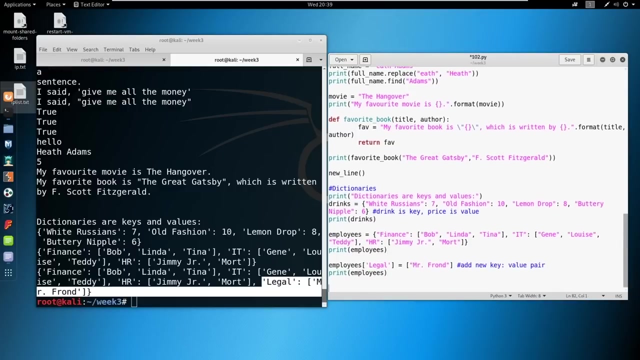 Hey White Rose, how you doing. Okay, so now, if we print employees, You can see now that legal has been added and Mr Frond is there. We could also use something called update Instead, so we could say employeesupdate and we could do this. 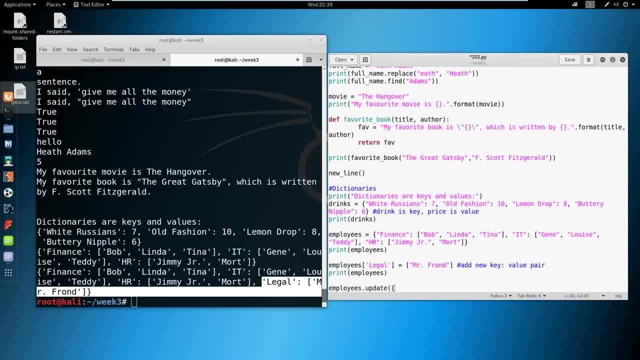 Let's say there's a sales department that comes in, right, We can say, okay, well, Andy and Ollie are going to be in charge of sales. And honestly, guys, I'm a bit saddened. None of you have picked up on the references yet, but that's okay. 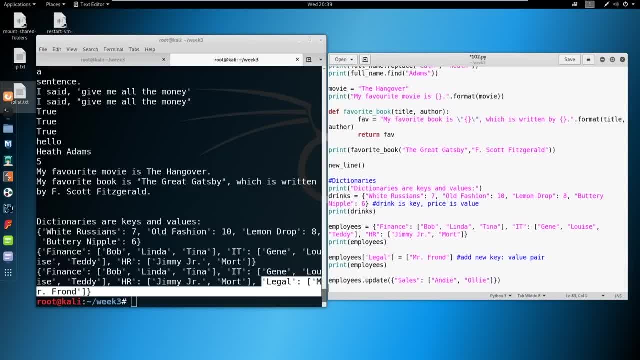 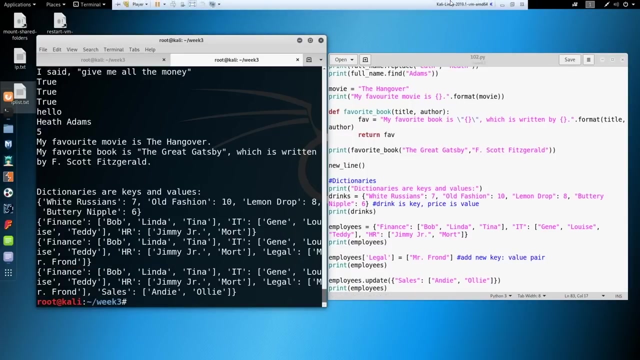 I will forgive you. Let's print out the employees again. This is not bake-off Man. we should have done bake-off. There's just not enough people on bake-off. I feel like This is all Bob's Burgers characters. 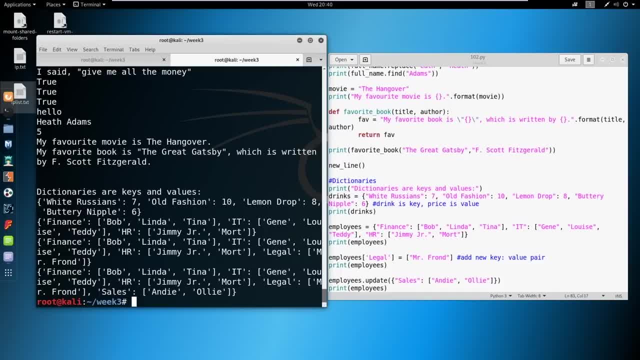 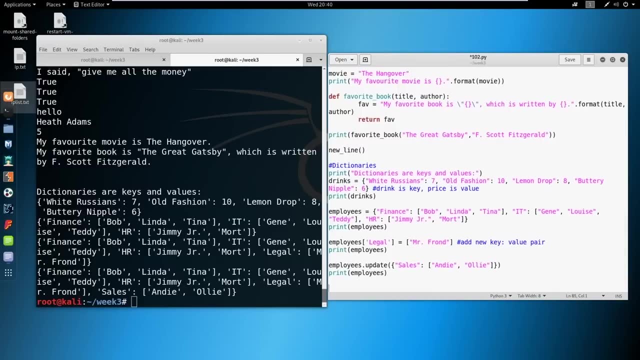 All Bob's Burgers. It's not friends Who said friends, All right. So you saw a couple different ways that we can add in. We can also update. So let's go back to the drinks. Let's say we wanted to update the price of a White Russian. 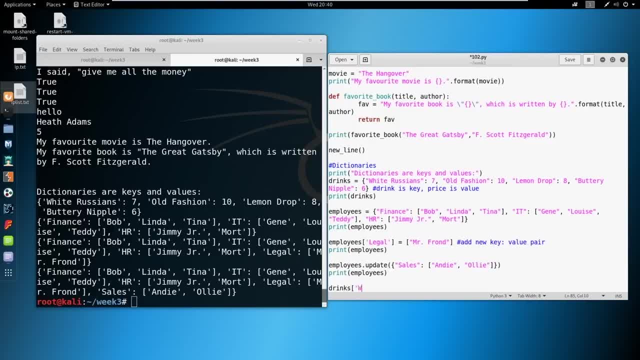 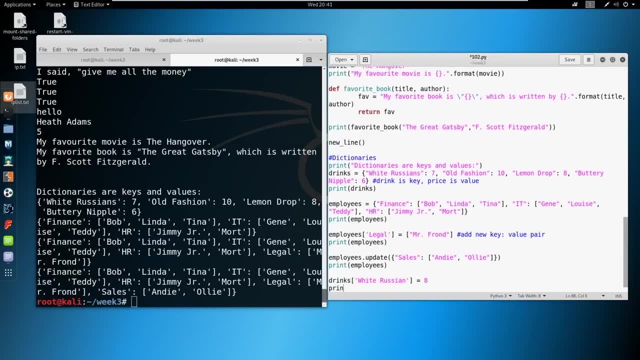 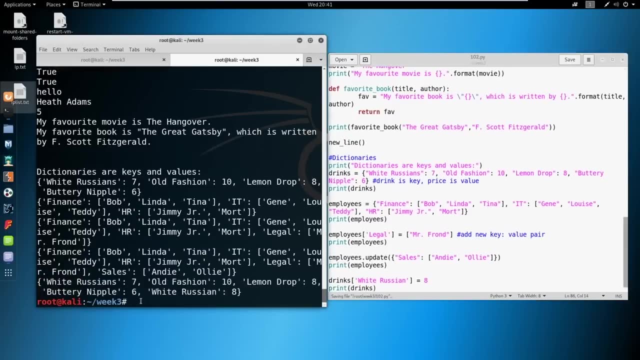 The White Russian is $7 right now. But let's say we want to make it $8.. We can just say drinks White Russian And just say it's equal to 8.. We print out drinks. You can see now that a White Russian is still $7.. 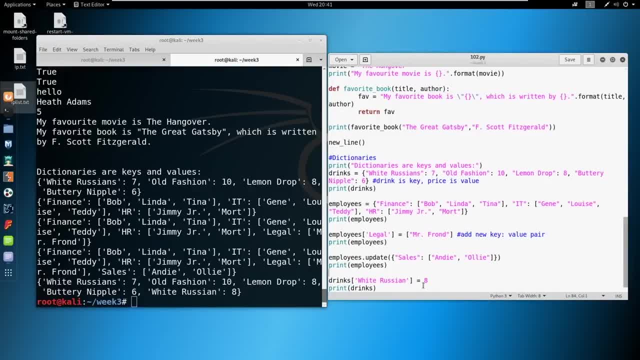 Why is that, guys? I literally have no idea. I literally have no idea. Other than this potentially hates me. Oh, I called it White Russians, White Russians, Huh, Huh, Yeah. Syntax is everything: $8.. 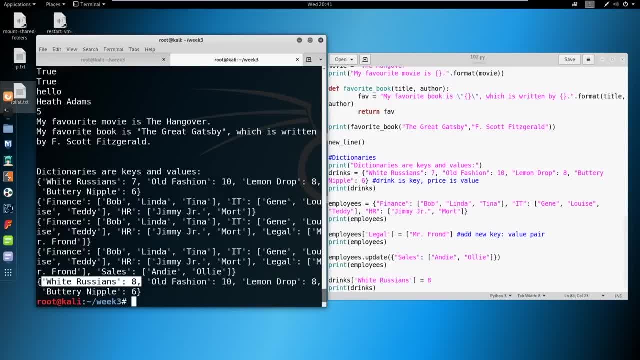 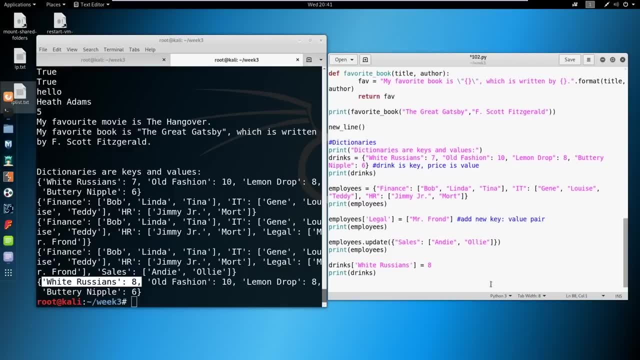 We just updated. Good job, guys. Extra set of eyes are important. All right, Let's say we wanted to know the price of a White Russian, but we didn't know how much it costs. We could say: print drinksget, Say White Russians. 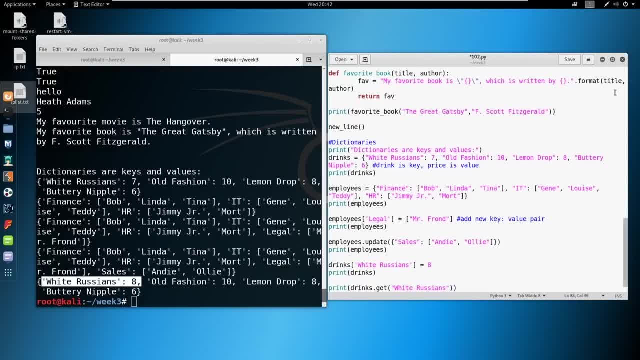 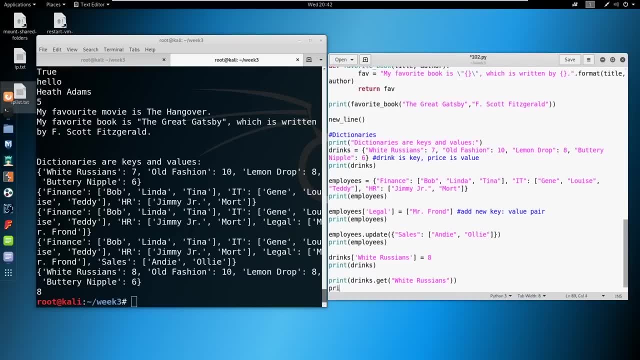 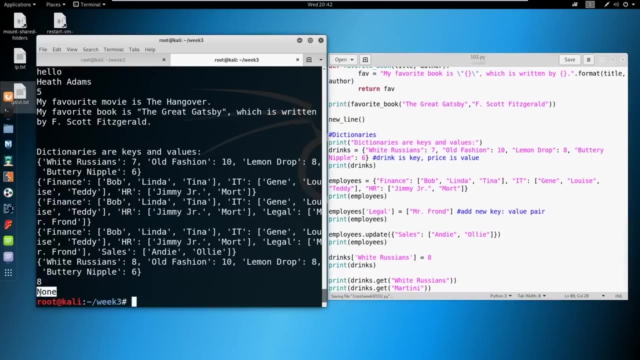 Don't know why I called it Russians. I'm sticking with it now, You'll see it returns $8.. What if we try to get a drink that does not exist? It'll return none, So it's good to make a note of that. 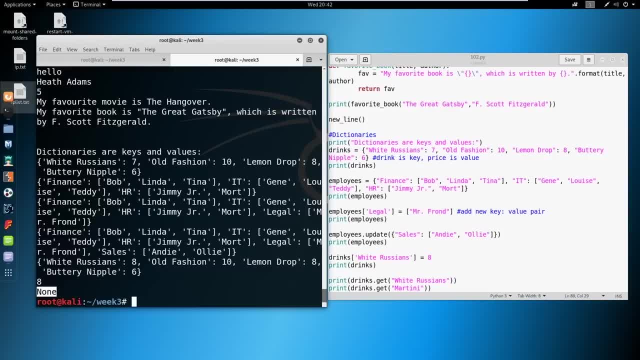 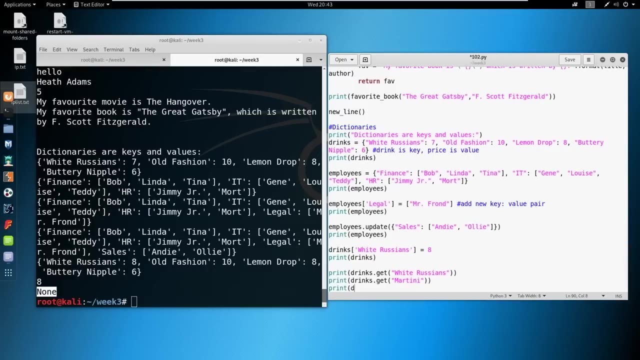 All right. Last thing I want to show you guys. So last week we took a list and we combined it up and we made two lists into one list, paired correct. JBL asked a question: Couldn't we just do print drinks, White Russians? 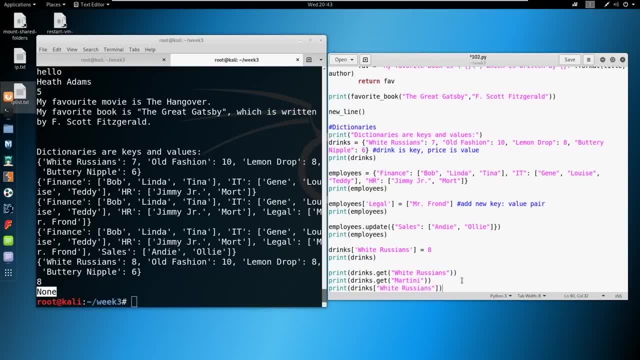 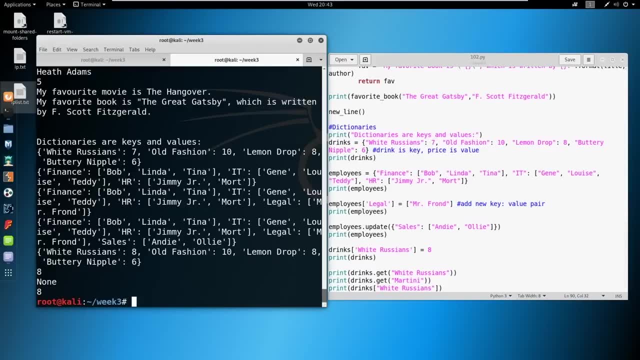 Yes, you can. JBL, Both work Okay. So we're going to do what we did last week, where we combined movies and people, But instead of putting them into a list, we're actually going to put them into a dictionary. 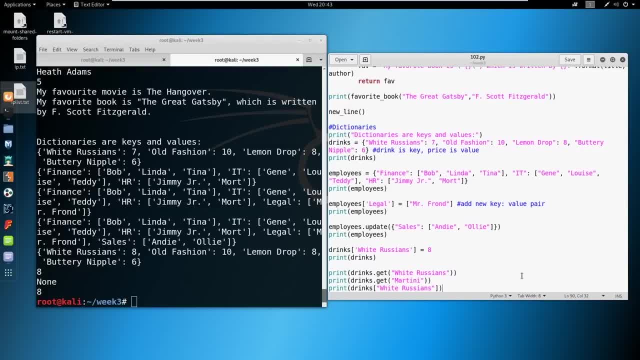 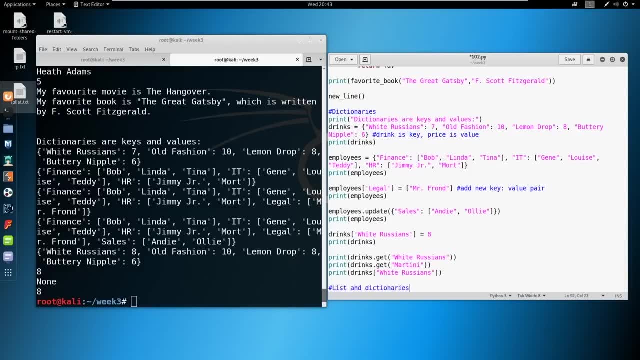 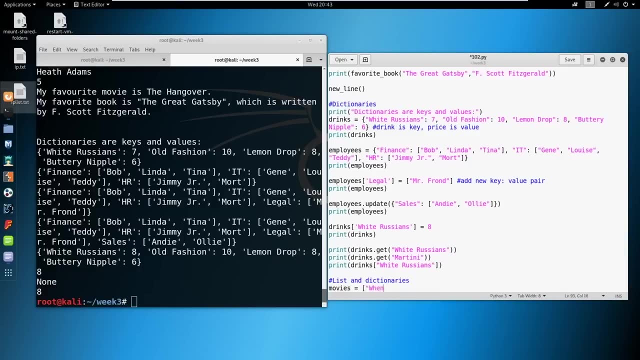 Very similar process And I will show you how it works. So we'll just call this list And dictionaries. All right, You can put whatever movies you want in here. I'm going to use the same from last week, So we'll say When Harry Met Sally. 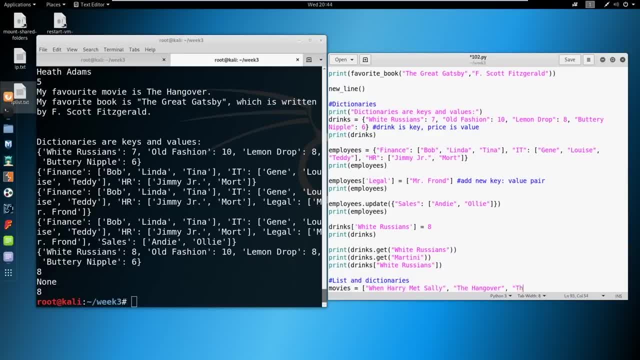 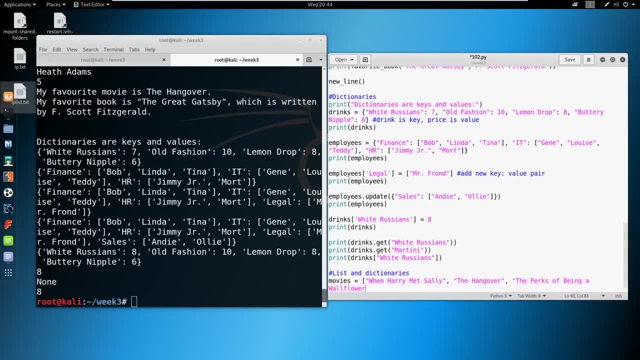 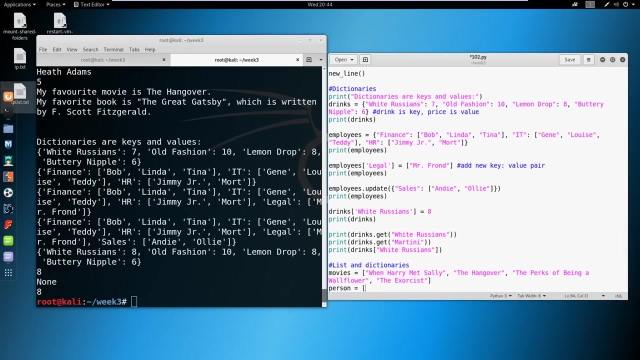 The Hangover Perks of Being a Wallflower. Wallflower And The Exorcist, The Exorcist Okay, And we put it to people right. So we said that I like When Harry Met Sally And say Bob liked The Hangover. 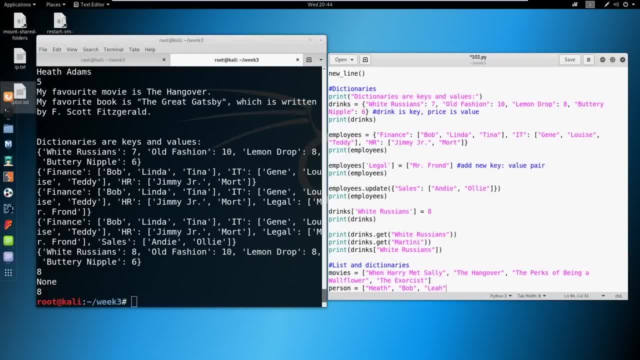 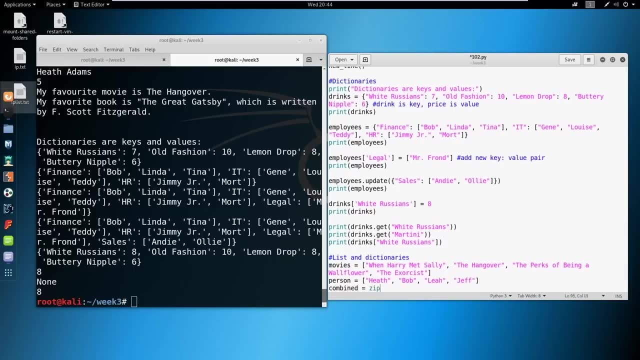 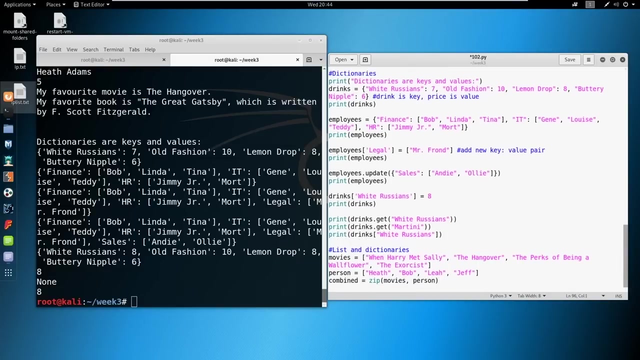 We know that Leah likes The Perks of Being a Wallflower And that Jeff liked The Exorcist. And then we did something similar. We said combined, And we zipped them together. right, So we put these two together And now, instead of doing what we did last week, 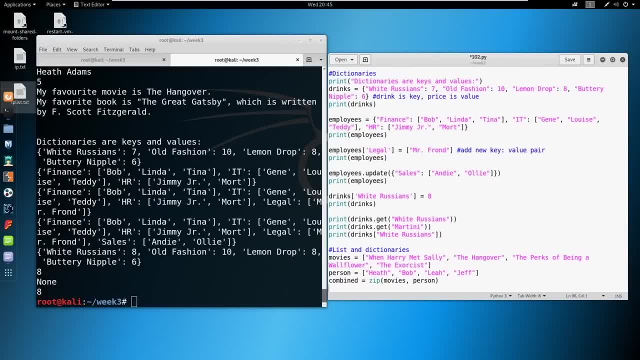 and printing out a list. we're going to make a variable here called movie dictionary And we're going to type this little syntax out here. So we're going to put it into a dictionary Like this And we're going to say key- value for key. 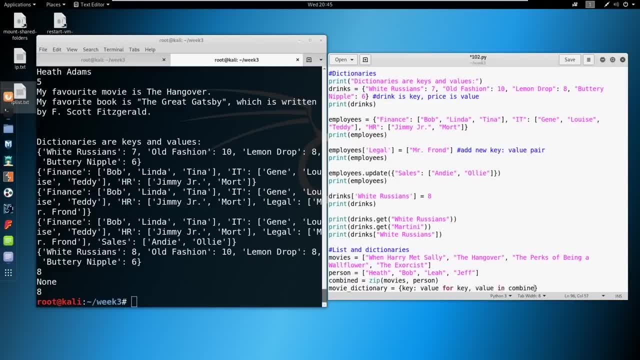 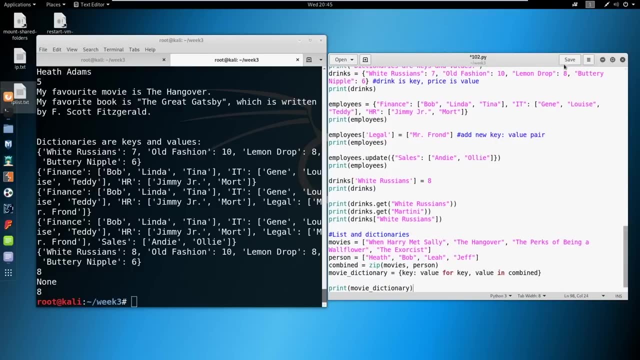 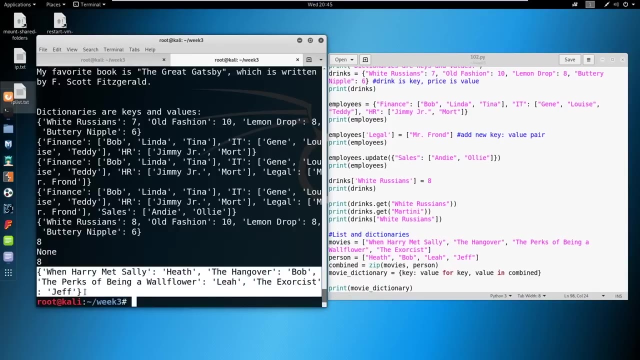 value in combined. Okay, Now let's look what happens when we print this out. And now you see we are in a dictionary instead of a list. We took two lists, combined them together and put them into a dictionary, So we've got lots of options in Python here. 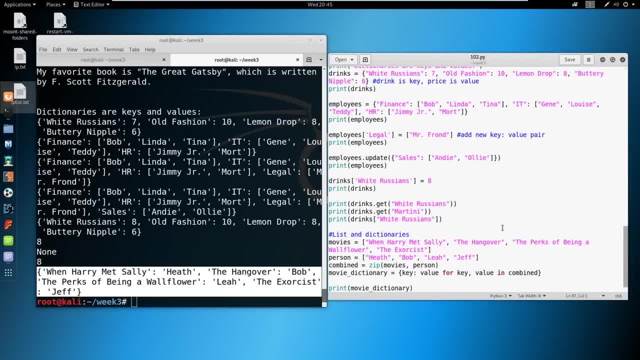 But without getting too advanced. I don't think we need to go any further. There's a lot more that we can do, But with the amount of time we have, I definitely want to build this shitty port scanner, And I want to show you a couple more things. 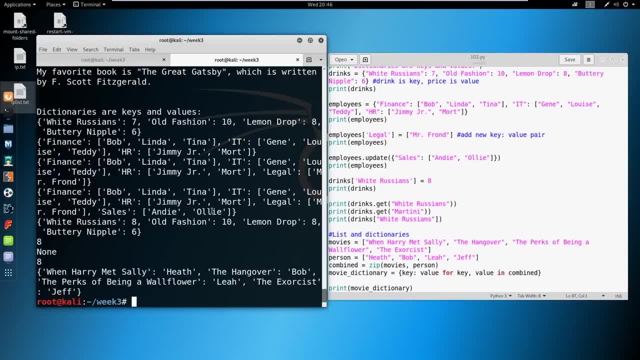 So one of the awesome things about Python and one of the things I use: if you remember, in episode one I showed you how to use system CTL. We talked about enabling a service. We worked on Apache right, We started an Apache server, opened it up on port 80.. 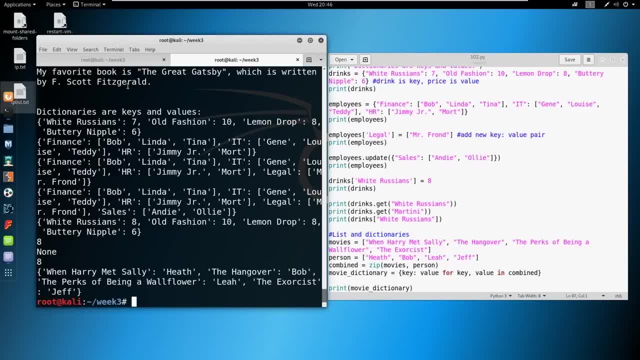 That's all great. The thing about the Apache server is you have to put your files into a var www folder, So everything that you want to specifically be hosted has to go into that folder. Instead, if we use Python, we can actually host a server wherever we are at. 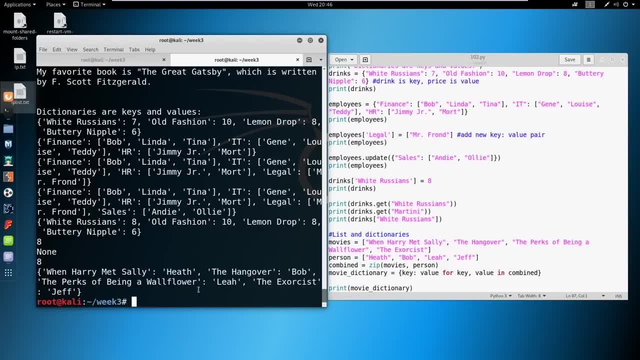 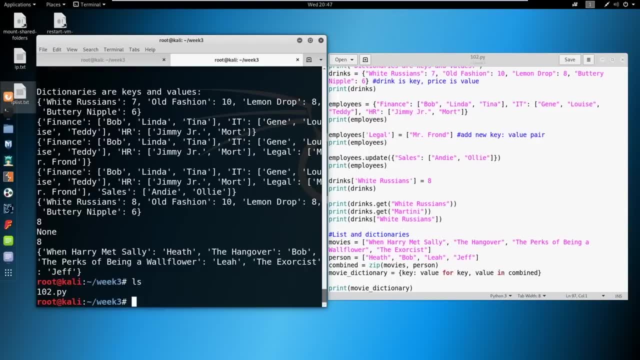 So let's take a look at this. Let's say, okay, we'll say ls, right, We've got this 102-py script. What if I wanted to host this? Oh, it is simple: HTTP server time You've got. 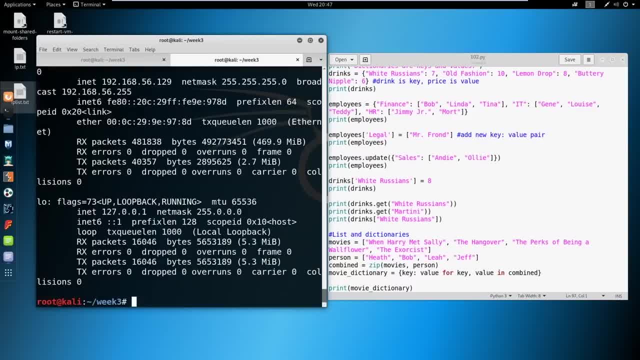 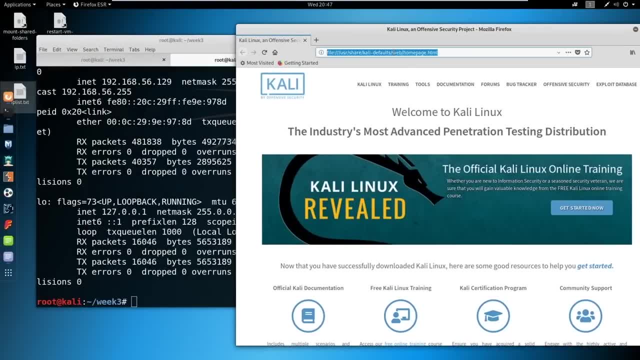 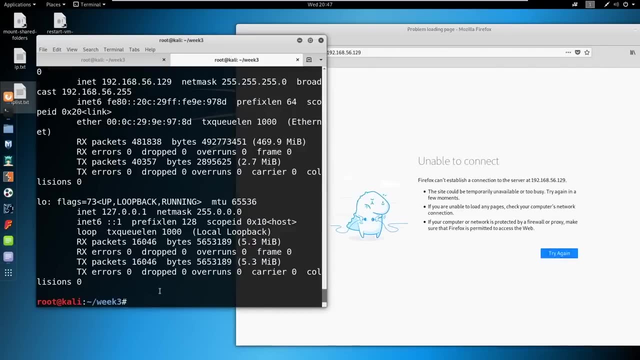 So I want to host this out on the web. Let's get my ifconfig And I'm just going to go into here And I'm sitting at 192.168.56.129.. Unable to connect, But I can just say: python-m- simple HTTP server, 80 for the port. 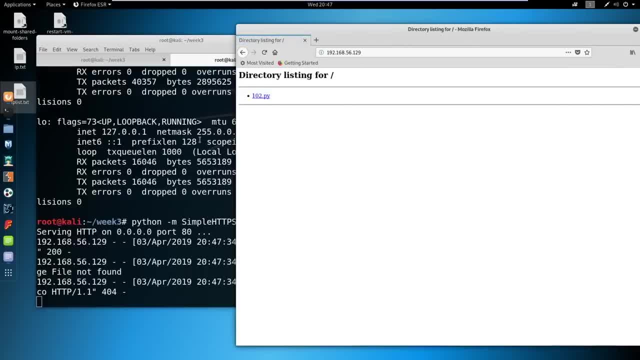 And if I come in here now, I've got a directory listing of everything that is in the folder that I'm hosting. So if I wanted to host up malware on a machine or get to some file to download quickly, this is a quick way to do it. 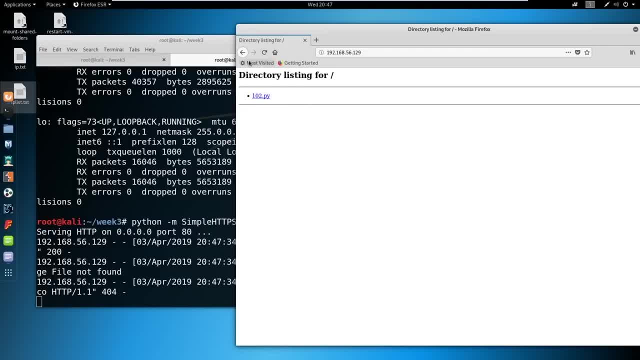 We'll talk about file transfers at a later time. This is one of my go-to techniques. There's many, many techniques. Linux is nice because Linux has wget, But when we get into Windows- Windows- you sometimes have to be crafty with your extractions. 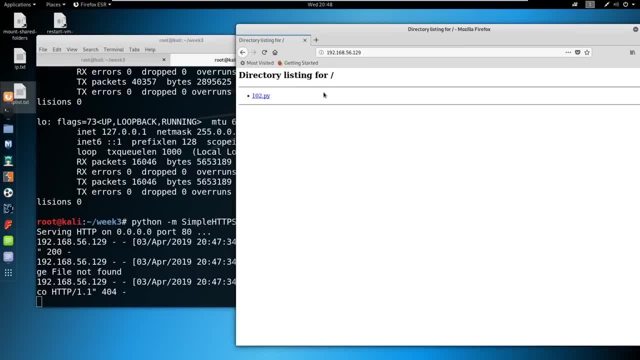 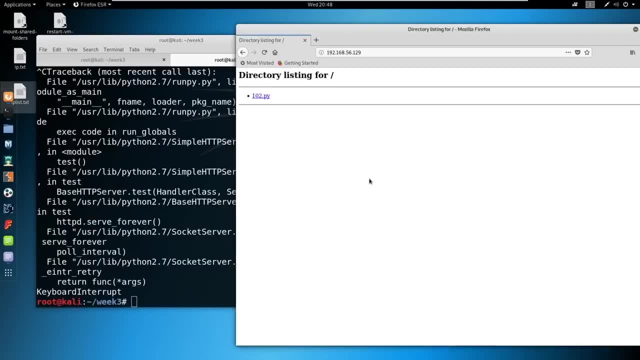 So we'll get into all the clever ways that we can extract files on a Windows machine when we get there. Now, this is actually the Python Python 2 method of doing it. There is a Python 3 method now which is slightly different syntax. 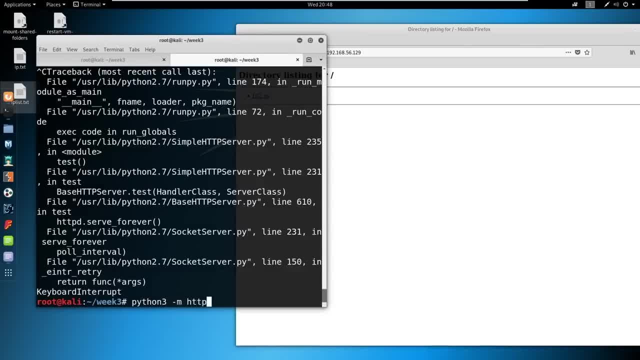 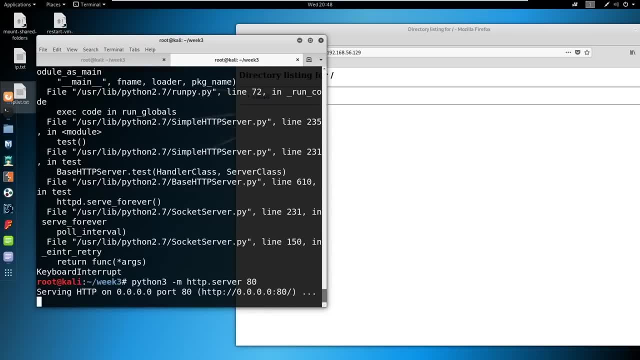 We just say python3-m and it is http-server80.. That is the only difference. You can host up whichever one you want. Both will work. But since we are doing all Python 3 lessons, I figured I would show you that. 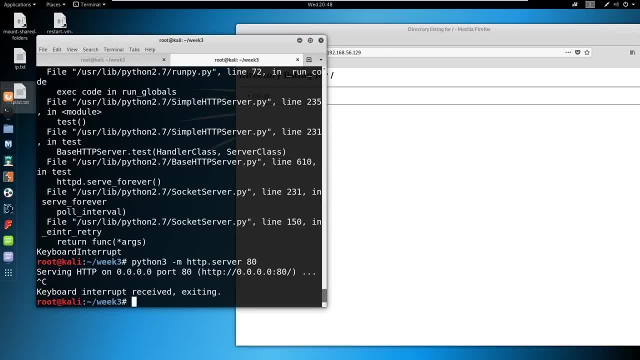 Now another way that is common to extract files on a Windows machine or send files over is to host up an FTP server. Now you can download an FTP server and make that work, hosting it up, transferring files that way. But another thing that we can do, 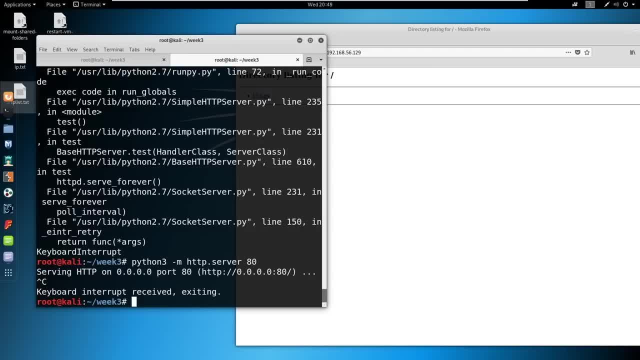 is, we can host it up with Python again in the area that we are in right, The folder that we're in. So this is called pyftpdlib. We need to actually install it, So we're just going to use pip. 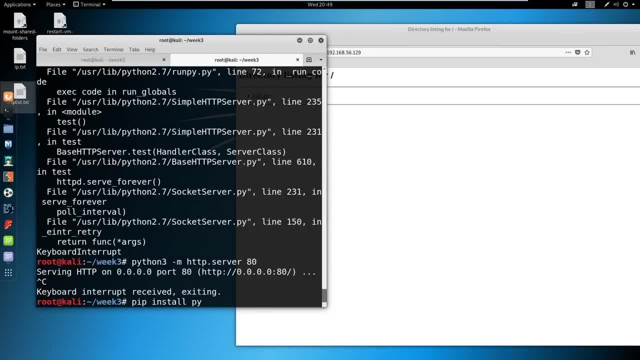 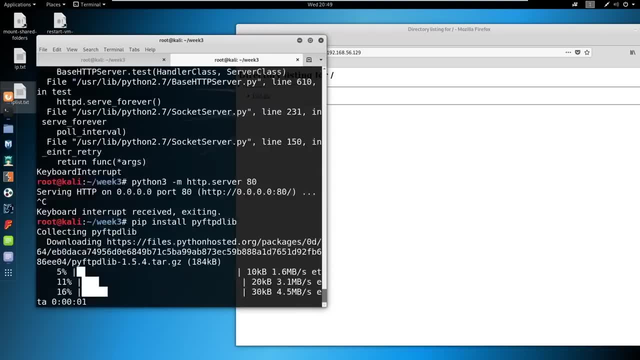 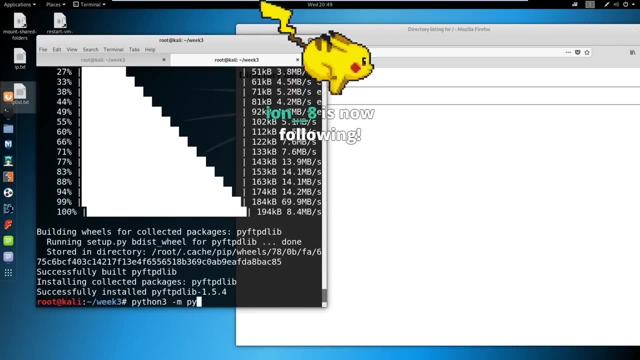 and install it, Or pip3, if you've got pip3.. Just type pip, install pyftpdlib. Okay, And then it's as simple as saying python3-m- pyftpdlib. Maybe, if it wants to work, 21w. 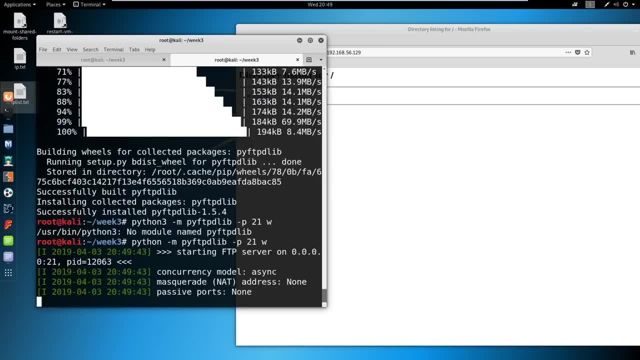 No module, Maybe for just Python. let's try it. There you go. We might need a pip3 install again to get it to work for Python 3.. So we won't do it twice, but just know. So now we're hosting up an FTP server. 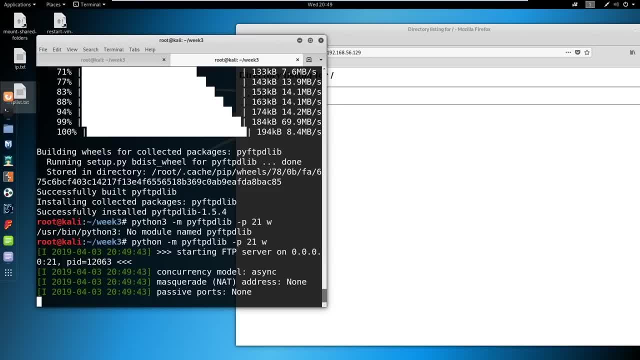 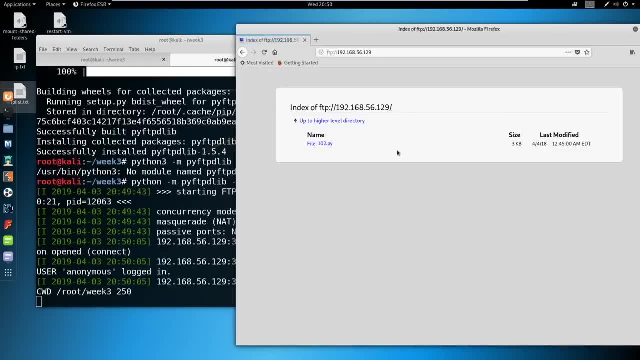 If you went onto a Windows machine, FTP is built in. You can transfer files. that way, If we said in front of this FTP like this, you could see that we've accessed this Because we put the W here. it should be a hyphen W. sorry. 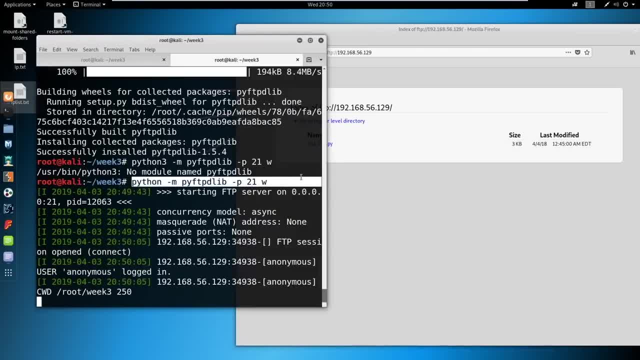 It's allowing log in anyway, but this should be for anonymous log in, just like this Worked with pip3 and python3 for Leah- Awesome, So I'm not spouting craziness. Okay, we close the connection and there you go. 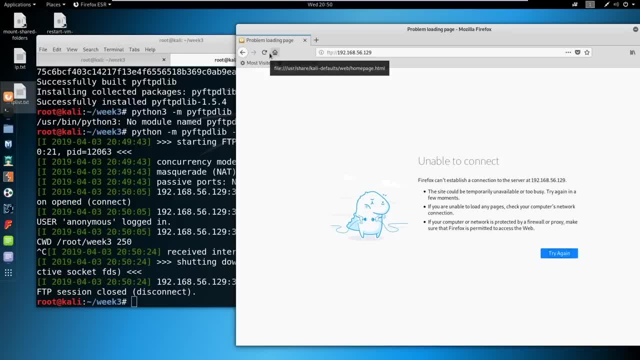 So you don't have to start a service and stop a service. You can literally just start and stop with control C in a quick Python module. So these are definitely important things. Ion, I see you. I will move your points over when I have a minute. 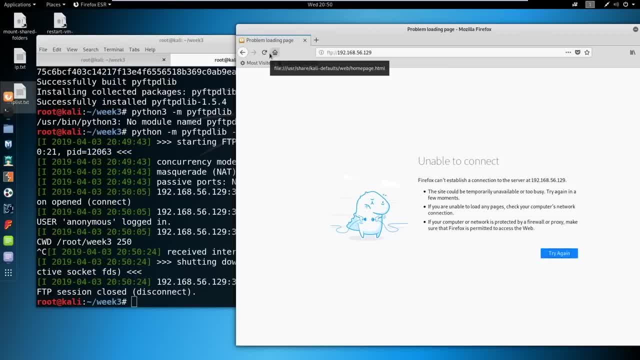 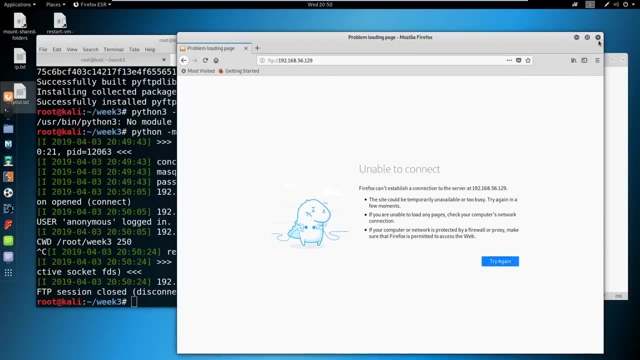 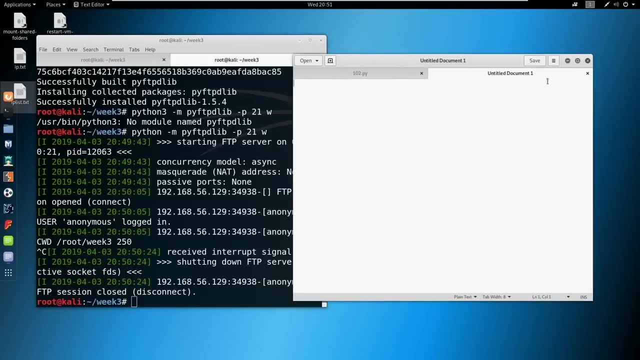 When we're done, before the giveaway, I'll move the points over. That way you have it. Okay, time to write our shitty script. So let's just do a new tab button here, And I'm going to go ahead and just hit save. 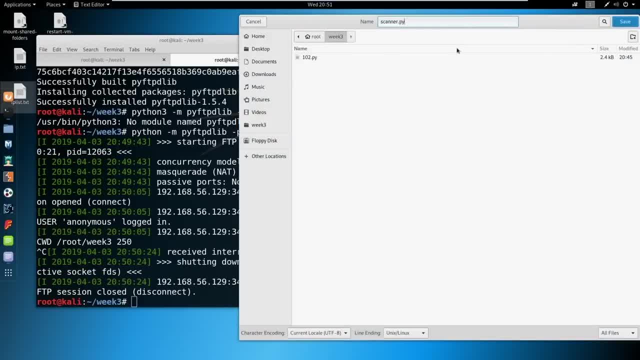 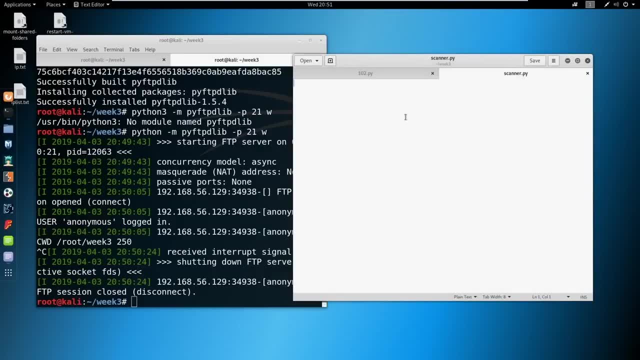 We're going to call this scannerpy And, of course, we're going to declare at the top: This has been Python three. Okay, so we really need to think this through on what we want to do. If we're doing a port scanner and we want to take arguments. 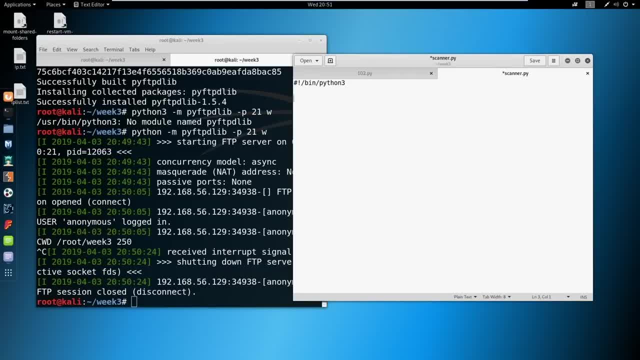 well, we talked earlier. Basically, if we're taking arguments, we're definitely going to need sys, right? So we're going to import sys. Hey Black Sheep, how's it going? We'll just say it allows us to enter command line arguments. 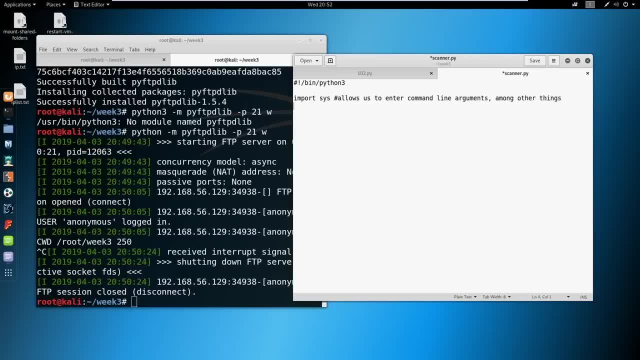 Among other things. it does a lot. There we go. We're not getting the fancy colors. Now we're getting the fancy colors. Okay, well, we also need to connect to a port, And while I haven't shown you this, 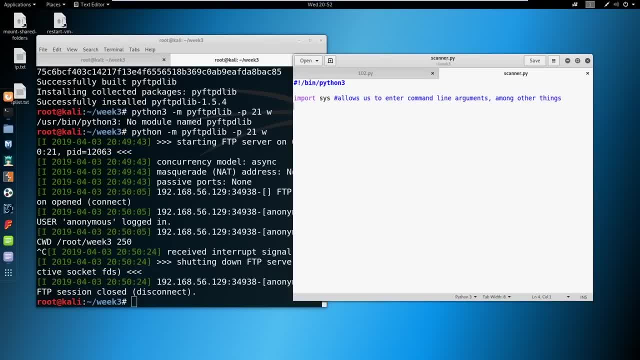 if you guys did your homework, let's see who did their homework. This is going to be a quiz. If I wanted to connect to AFInet or SockStream and I wanted to do a IP and a port connection, what am I importing? 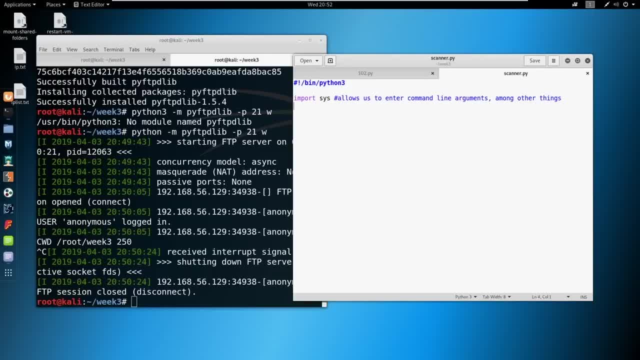 Who did the homework. We're importing Socket. Thank you For the rest of you. don't skip leg day. You need a good foundation and you guys are skipping leg day, Just saying, All right, we need to import Socket. 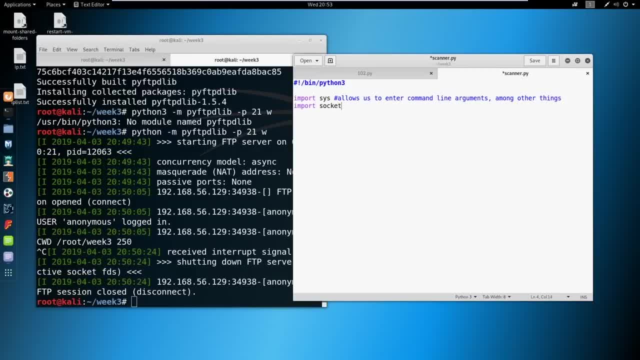 Thank you, Jeff. All right, And you saw this earlier. I want to add a little bit of pretty, So we're going to take some pretty and just add in date time. We'll import that Now. I will caveat that this script is stolen and modified. 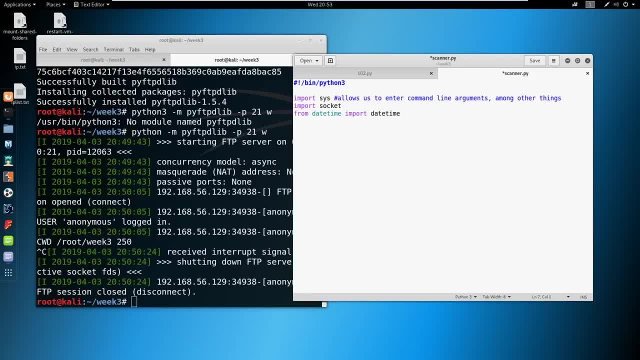 It has been stolen and modified all of the internet, So I have no idea who the original owner is. I'm just clarifying that this is definitely stolen and I have modified it from Python 2 into Python 3. And I've also 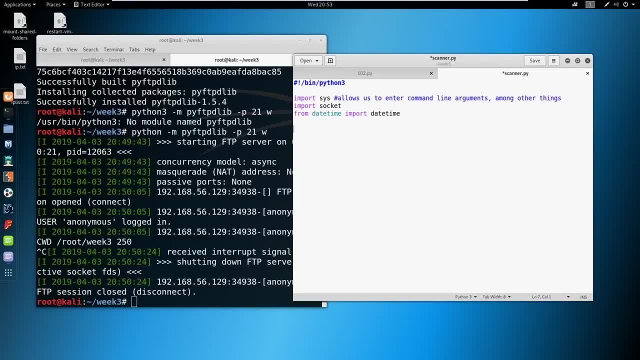 I've also changed some things, So I've made it my own a little bit, but the base foundation is definitely somebody else. I feel like my dad just told me he's not mad, He's just disappointed. Yeah, I am disappointed. 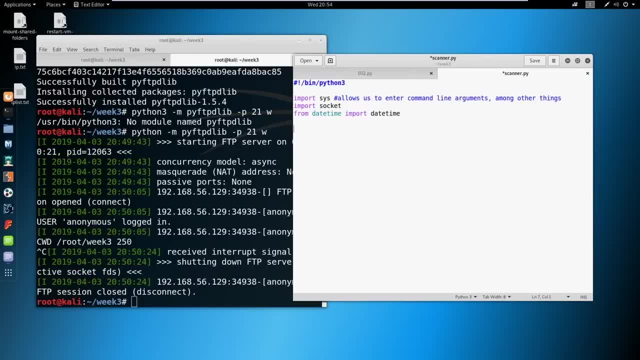 Do your damn homework, All right. So let's go ahead and set up our first argument, and we're going to define our target. Okay, so let's think this through. I'm going to take an argument, And when I say that, we have an argument. 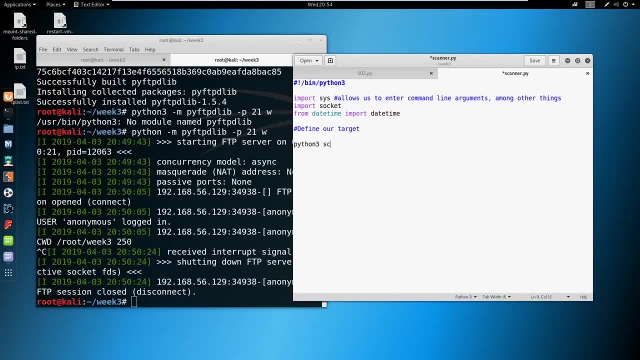 what I'm saying is when I write in this script, we're running Python 3 scannerpy. Now scannerpy is considered argument 0.. If we wanted to enter an IP address here, this would be argument 1.. This would give us a total of two arguments. 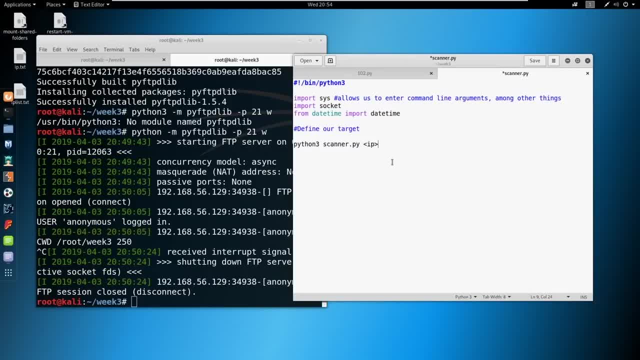 Remember we start counting at 0.. Now, what is some sort of statement that we'll need that checks for this? Do we know? Like what are we checking for? What would be something logical to check for here? And we're not going to make a perfect script- 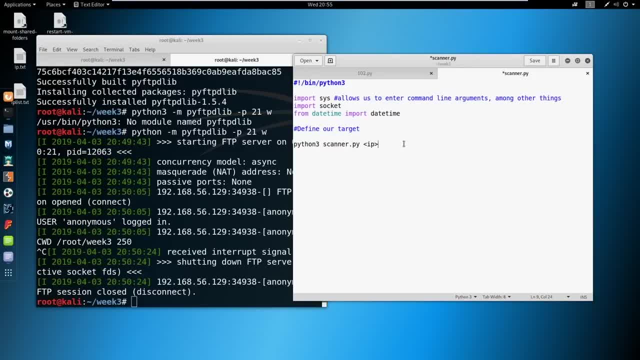 Remember, this is a shitty script. If argument 1 is empty or not, that's pretty close. That's pretty close. I'll do you one better. What if we say: are there any arguments? That's good. Yes, so we're in the right line of thinking. 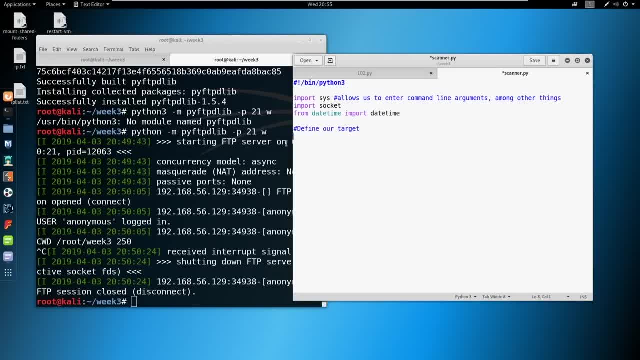 And that's really where I want you guys to be. I want you guys to be thinking logically, even though you don't know the syntax, thinking logically about how we can write this right. So we're going to say: if the length of the arguments argv. 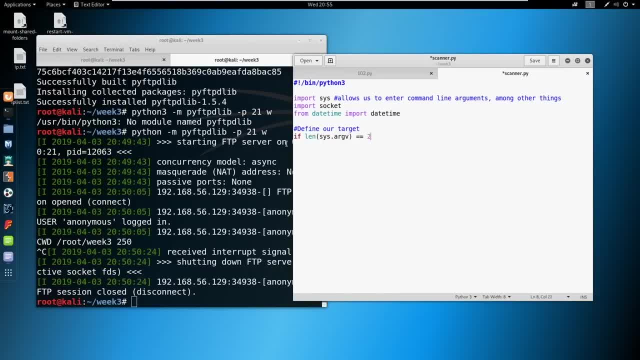 is equal to 2, then we can declare a target right. So this will look something like this: We'll say target, We'll call socket And we'll say: get host by name sysargv1.. And we're going to say: 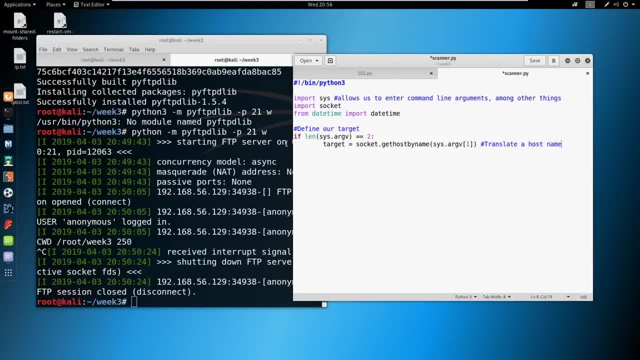 all this does is translates a host name to ipv4. If we need to. So if you have a host name out there, like one of my machines is called Punisher, If I entered Punisher, it would do a name translation and just put it into an IP address. 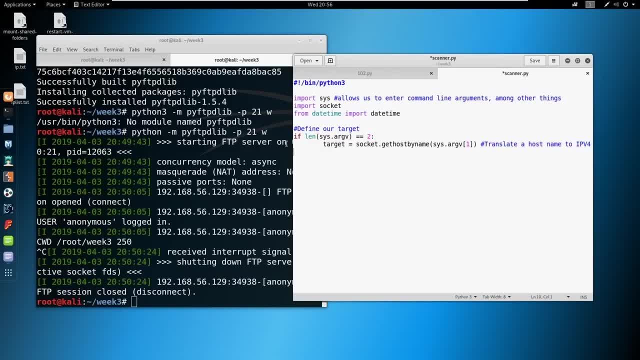 In theory, that's what socketgethostbyname does. Now, sysargv1 is the IP address that we want. So we don't want three arguments, We don't want one argument, We want two arguments. Now, this isn't going to be perfect. 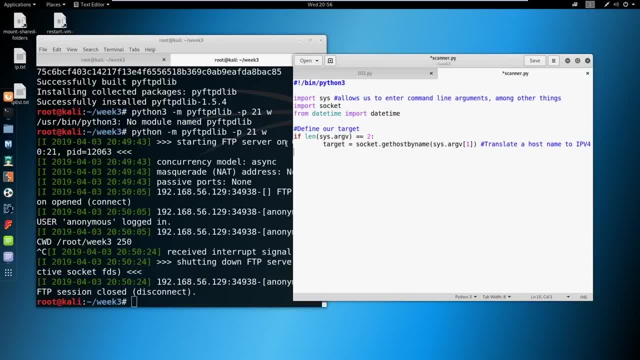 Remember, this is a shitty, shitty scanner, So we should be making sure that the arguments we're entering are a valid IP address, right Like we want to make sure that we're entering in, you know, three, three, three, three for each octet of some sort. 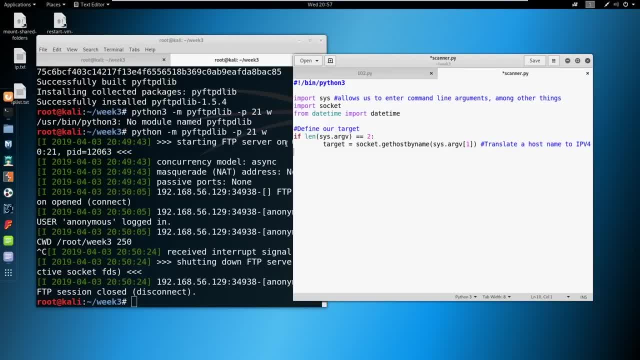 So now let's say that, okay, if our length is two, then we're going to go ahead and set a target based on what we input. So we're going to input for sysargv1.. If it's not two, we're going to print out. 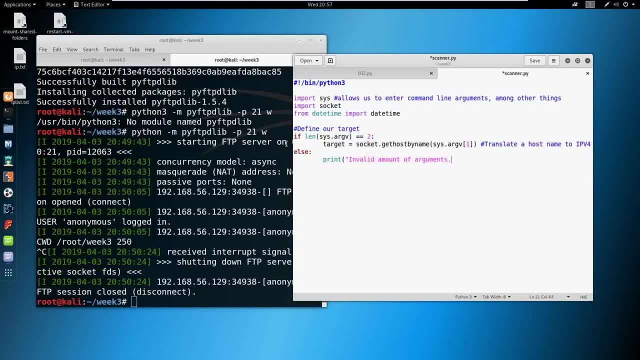 invalid amount of arguments. And then I like to generally give out syntax, So we'll say syntax, python3, scannerpy, IP And most of the arguments that we're going to use, most importantly sysexit, which allows us to actually close the program. 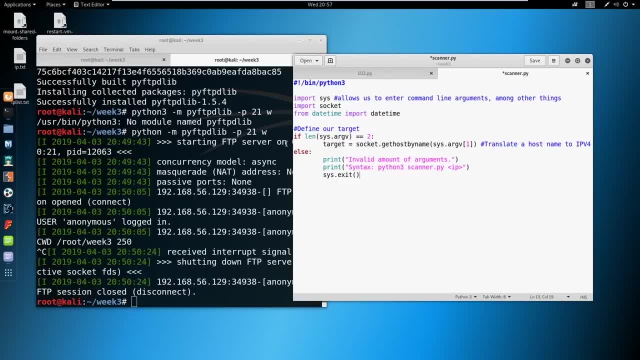 If you don't sysexit, it'll hang. So this will exit for us. So it's always good to check your work as you go, So I'm going to go ahead and do that now. python3 scannerpy. Okay, I didn't put in an argument. 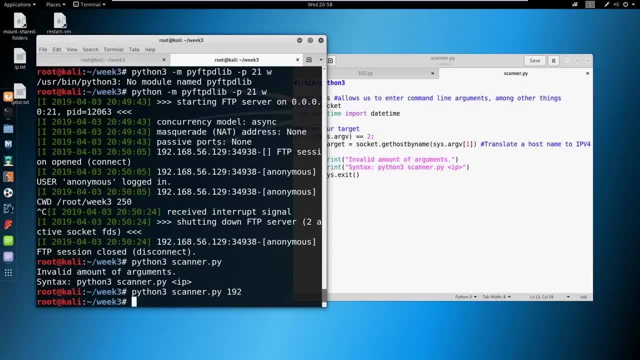 And now I'm going to put in 192.. And it doesn't throw any errors, right? Can you control C? if you don't, sysexit, I think it hangs without a control C. Let's see I could be wrong. You're testing my knowledge here. 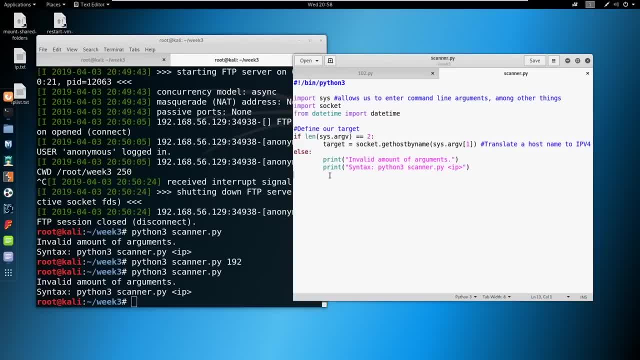 Actually, it worked fine. I think what's going to happen is, when we start adding more arguments, it's going to hang Or it's going to try to move on to the next thing. It'll keep reading the script And what we're doing is we're actually exiting the script. 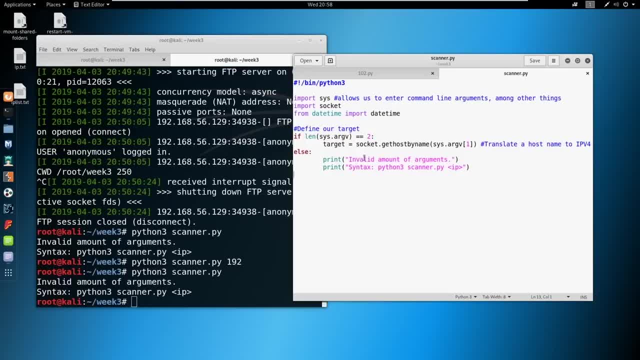 at this point. if that makes sense, So let's go ahead and throw that back in there And let's add some pretty. We'll say, add a pretty banner And we'll put in times 50. And we'll print Scanning target plus target. 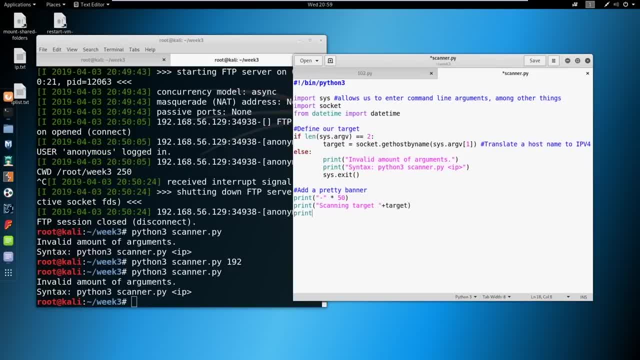 We could also use a placeholder here. Print times started And we'll say plus string of date time dot now. Remember we have to convert to a string to put into the string: Close that, Close that, Close that. Three of those. 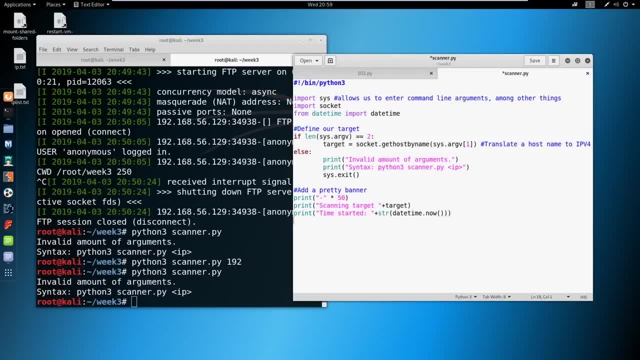 Banner's top priority. You want to do ASCII art the rest of the time? I agree. actually, We'll print another 50 here of these little dashes, And that should give us a pretty little banner. So here's where we can test it out, right? 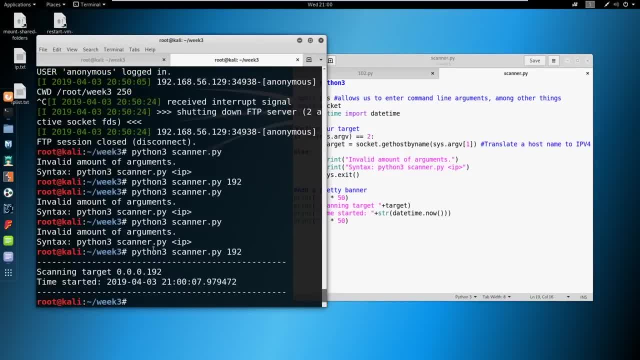 So let's say we put 192 right here, You'll see, it tries to convert into the correct subnet And it prints out our cute little banner, our pretty banner. Now let's take out the sys exit, just for demonstration. If we save and we throw no argument. 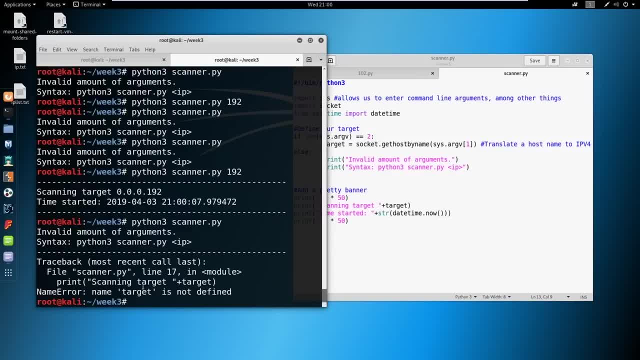 now we have issues Because, remember, we called target here. So it's trying to run through here and call target, But target's not defined because the length isn't set to two. So because we don't exit here, it tries to continue on and do the script. 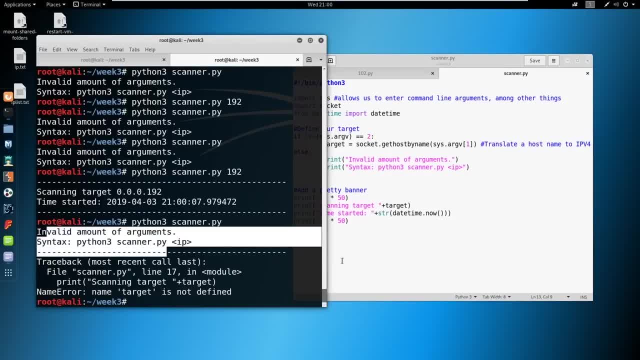 You see, it prints out everything. So this is why sysexit is important. Okay, I need a drink. I've been talking for way too long, All right. So now we're going to do a few things. We're going to use a try-except. 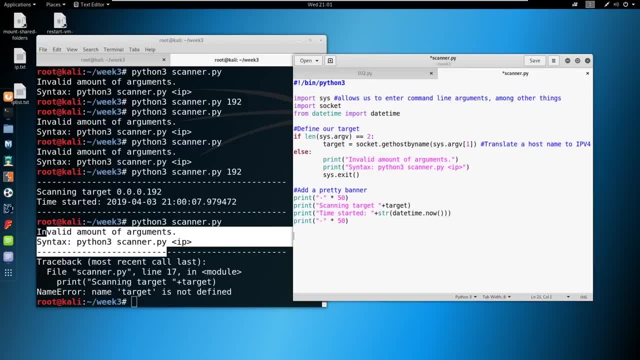 I showed you guys try-except last time, meaning we're going to try something and if we throw an exception of some sort then we're going to close out of the program. Bye, White Rose, Thanks for joining us. So we're going to say try. 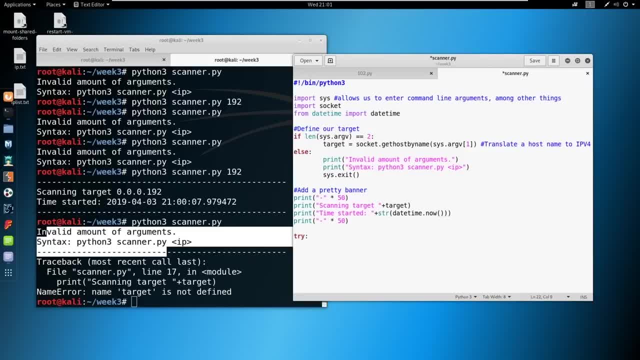 We have to indent on the try. Okay, So we're going to write a loop here. If we think about it, we need to grab ports. If we were making a not-shitty port scanner, we would probably want to be able to define ports. 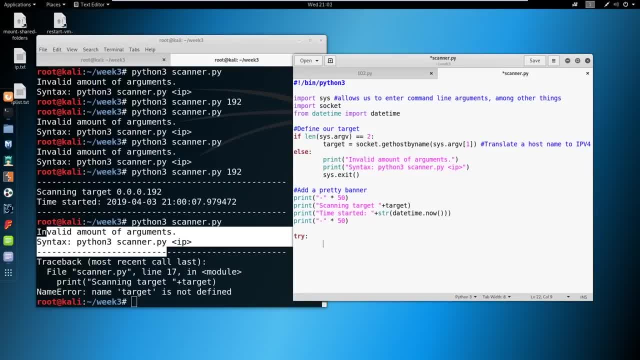 using something like R2.0.0, like arg-parse- Remember we saw arg-parse last time. We would import arg-parse and try to use that and try to make it better in terms of we can define it or if we don't define it. 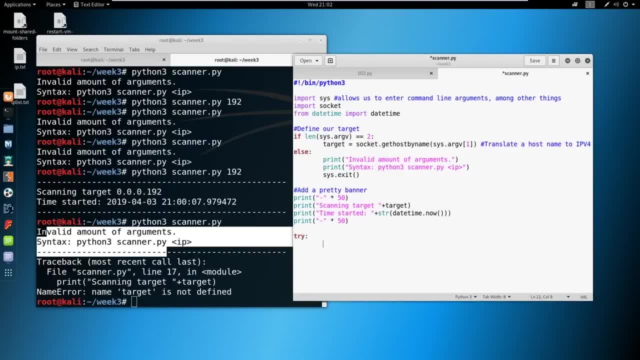 then it'll try to run through the top 1,000, kind of like nmap does. Otherwise we're writing a shitty port scanner. so we're actually just going to pick a range because we're not going to do threading or anything else. 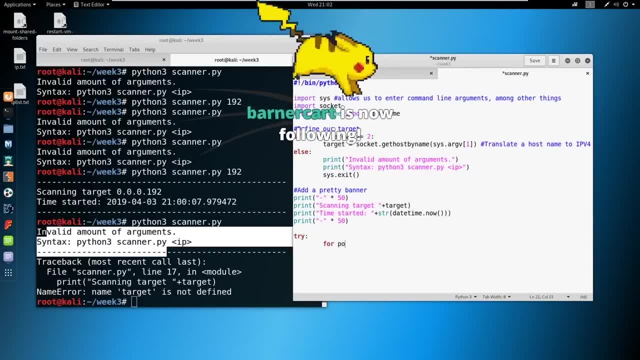 You'll see what this looks like. So we'll say for port and range, and I'm just going to define 50 to 85.. I'm going to scan my router and hope that port 80 or port 53 is open for DNS. 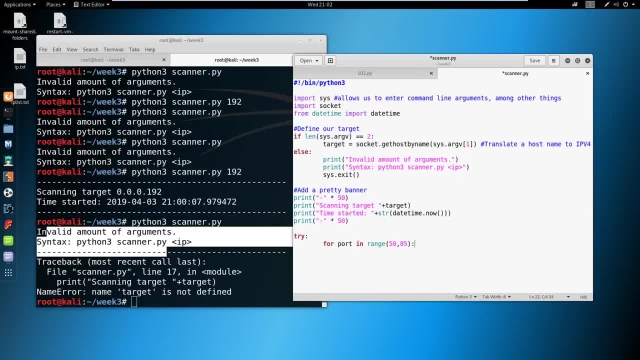 and you'll see why: because this port scanner is shitty and slow. We'll talk about that in a minute. So S equals: We're just setting a variable here, so we don't have to type this out every freaking time. This is very, very commonplace if you did your homework. 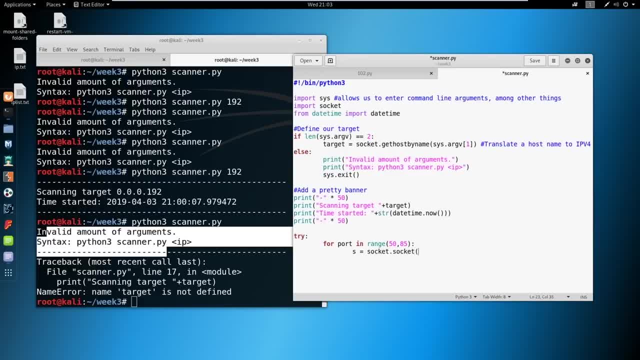 which apparently one of you did. S equals socketsocket, socketafinet, socketsockstream. Now, afinet is IPv4.. Sockstream is your port, If you've watched the videos on the buffer overflows that we've done. 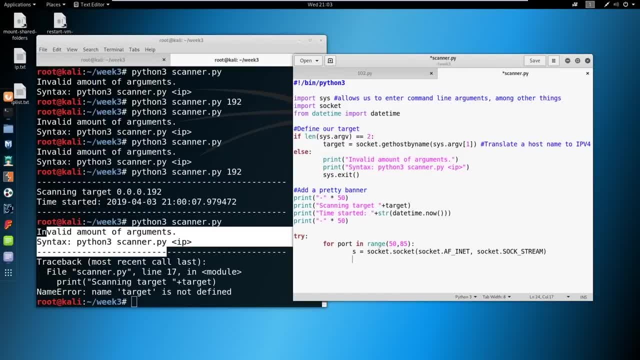 that's all it is, So you will have seen that previously. Hey Barner, thanks for the follow. We are doing Python lesson this week. This is a hacking course overall, though, So we're going to say socketsetDefault- Timeout. 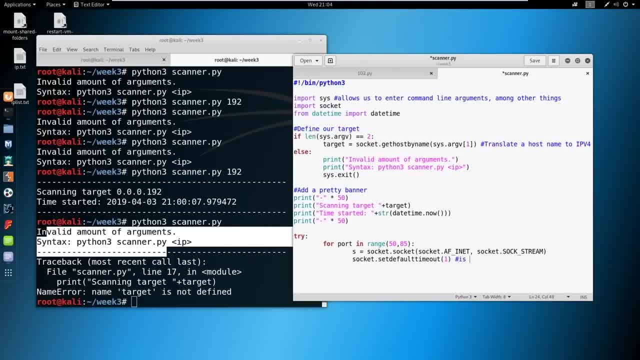 I'm going to put it to one second, but I'm going to note for you guys that this is a float, So we could put in here 0.5 if we wanted to. We'll just do one second, But basically, if it doesn't detect that the port is open, 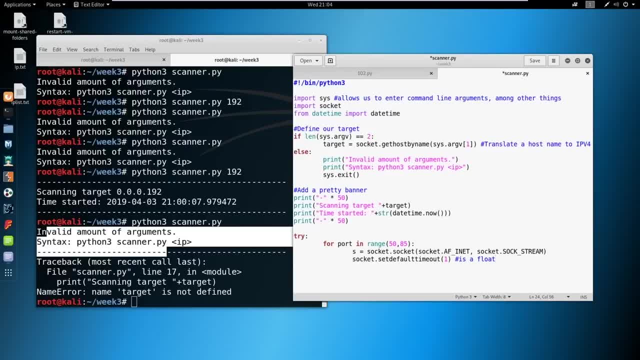 then it's going to move on after a second, or else it'll hang forever. Okay, and then we're going to restore our results In sconnectex And we're going to say target port like this, And all this does is this: returns error indicator. 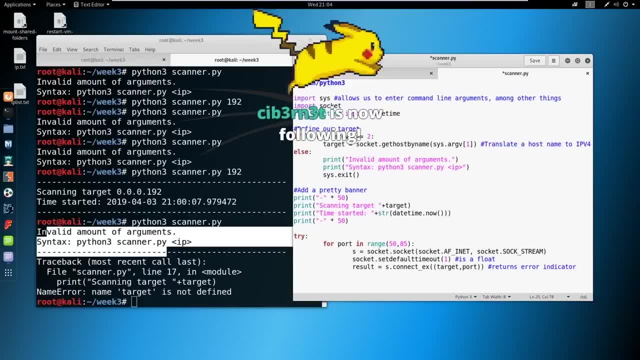 So if there is an error on connection, it'll return an error indicator. If there is no error on connection, it returns 0.. So, with that being said, we could print out: if result equals 0, then we know that we were successful in connecting. 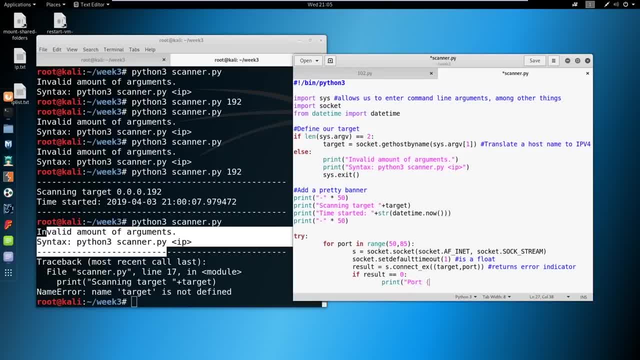 And then we can just format that here with port, And then we'll close the connection. Thanks for the kind words, Barner. I appreciate that. Okay, so I'm going to add in one thing here, just for proof of concept. Typically we wouldn't leave it in. 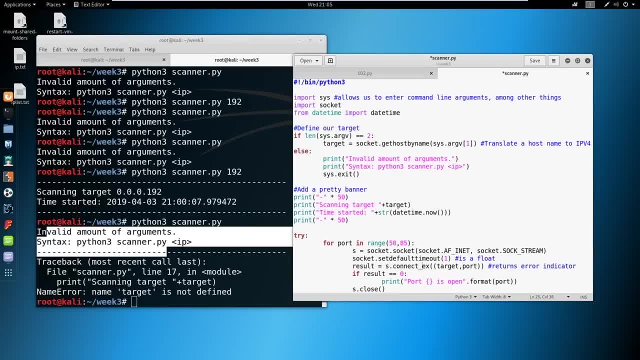 and it's going to spam us a little bit. But I want to add in here that we're checking the port. Okay, So we know that it's actually running. Okay, so let's talk this through. So we're going to run a for loop. 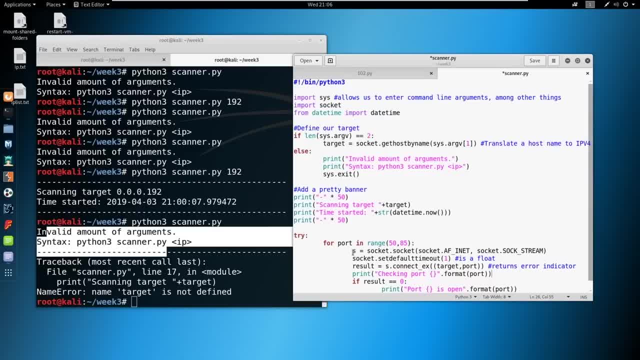 So for every number between 50 and 85, we are going to set up this connection right here, We're going to define the variable, which is just this connection variable. right, We're going to set a default timeout of a second. 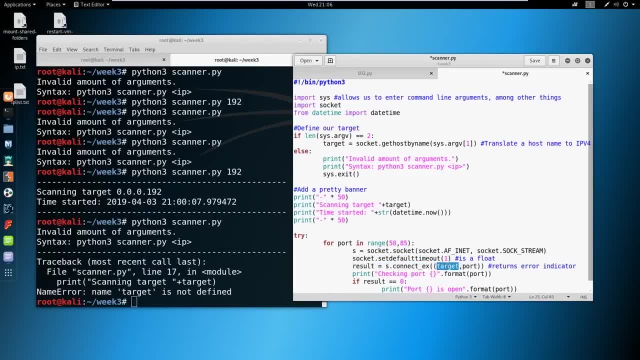 We're going to store our results. If we return an error on this connection, remember sconnect. So this is why we store this, because it would be socketsocket, all this in front of connectex And we're going to say target port. 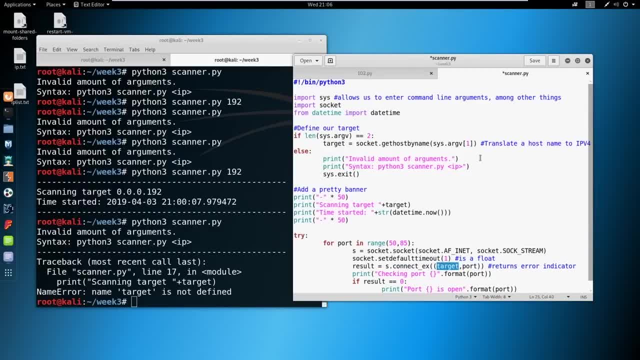 So we're going to take the target that we declared up here in our IP address. We're going to take the port that we're declaring here in this for loop, put it through here every time. It's going to return our error indicator. 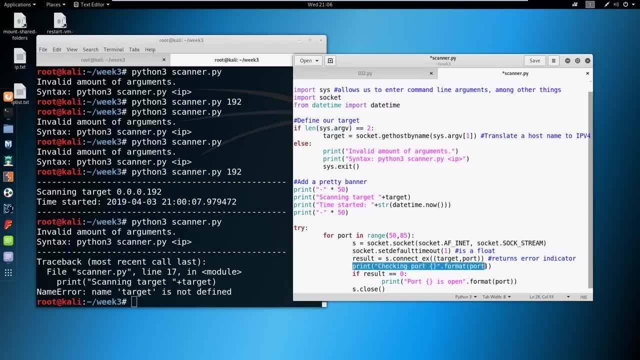 Before we do that, we're going to print checking port. We could do that before the connection. We could say it up here if we wanted to, instead of having it down below. It doesn't matter where you put it. And then we're going to say: if the result is zero. 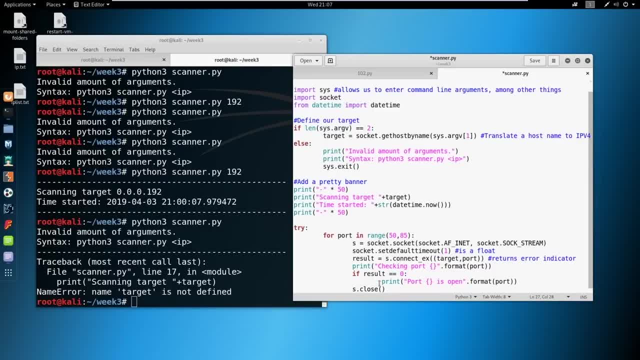 meaning that it is a success. we're going to print: the port is open. We're going to format that port just so it fills in there, all nice, And then we're going to close that connection, that particular connection, we're going to close. 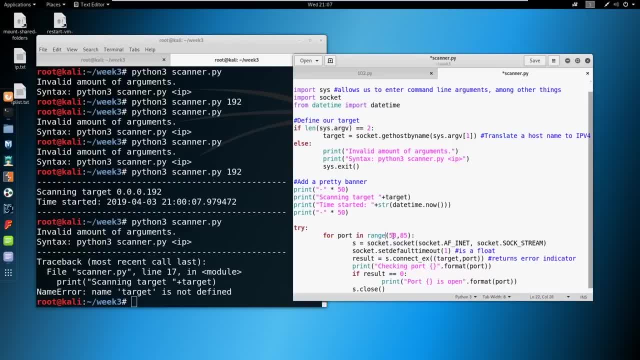 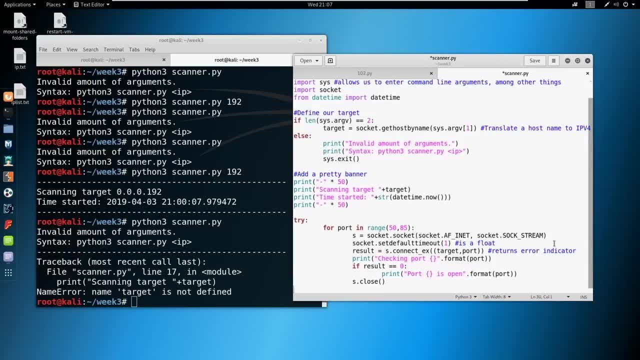 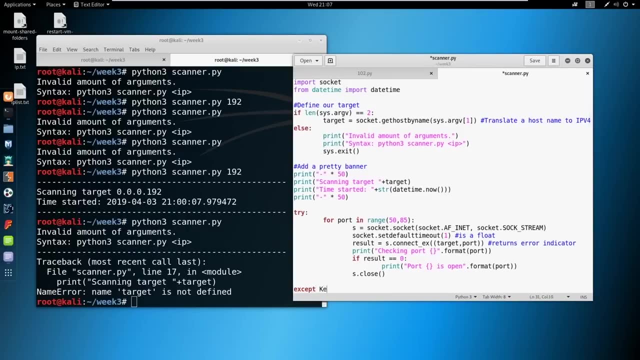 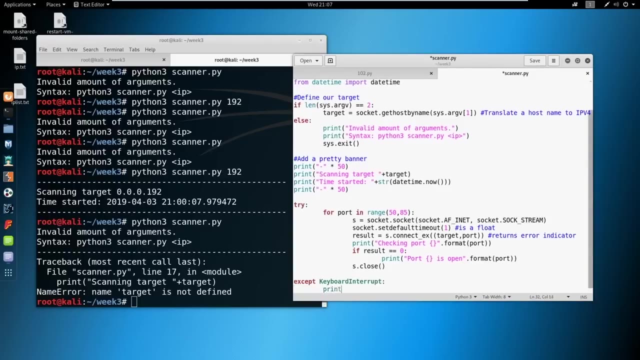 We're going to run through this whole thing however many times- 50 to 85.. Okay, Let's declare some exceptions real quick. So a few things I want to declare. So we'll say: except keyboard, interrupt, And then we'll just print. 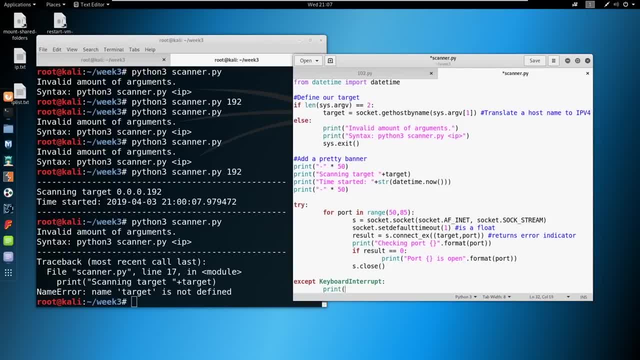 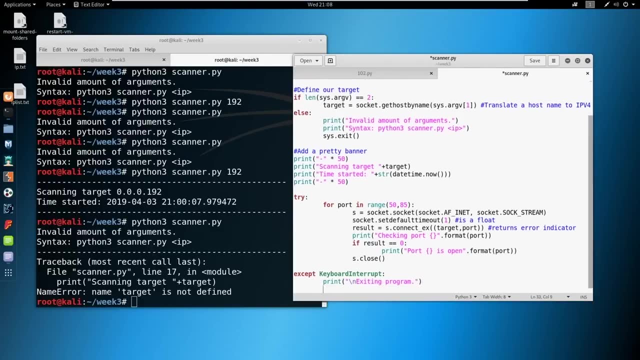 Make sure we add a new line here and say, oops, We'll say exiting program. So that way if we hit control C we can exit the program. It'll tell us we've exited the program. And of course we need to say sysexit, as we've learned. 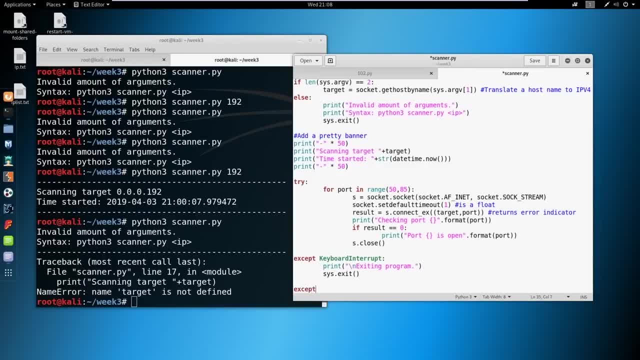 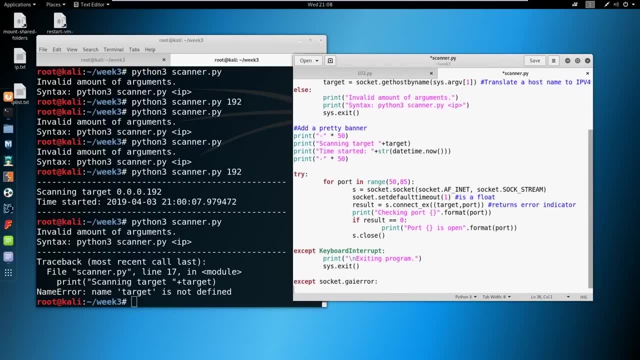 We're going to throw a couple more exceptions If the socket GII error, meaning that we cannot connect to the host name. did I forget a colon? Where did I forget a colon You tell me? I'll go back and fix it. 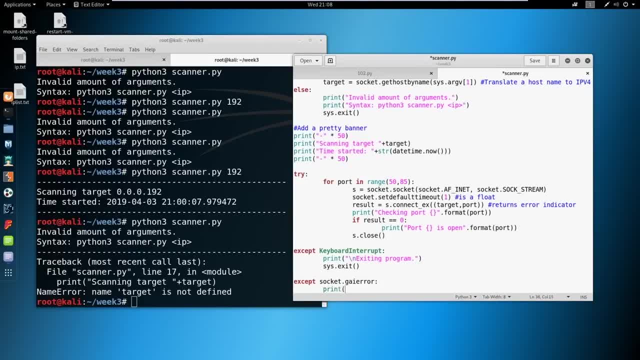 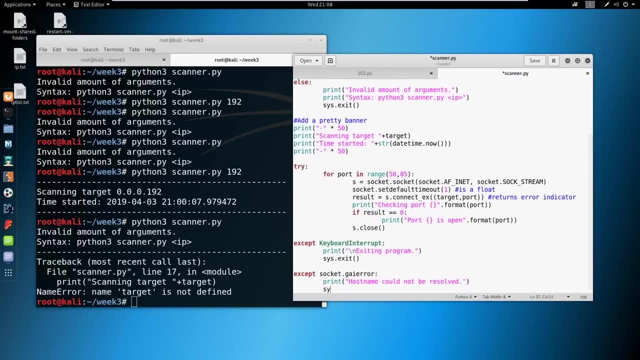 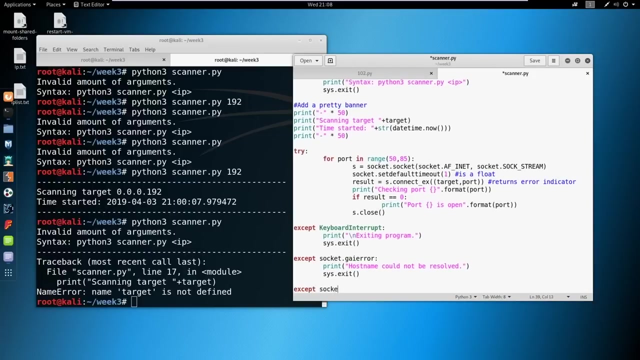 because I probably did So. if we can't resolve the host name, we'll exit out. And lastly, we've got the colon for, except It comes after keyboard interrupt. If we can't connect at all to anything, say the server is down. 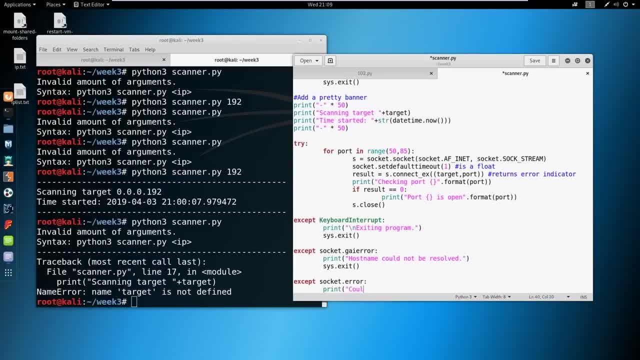 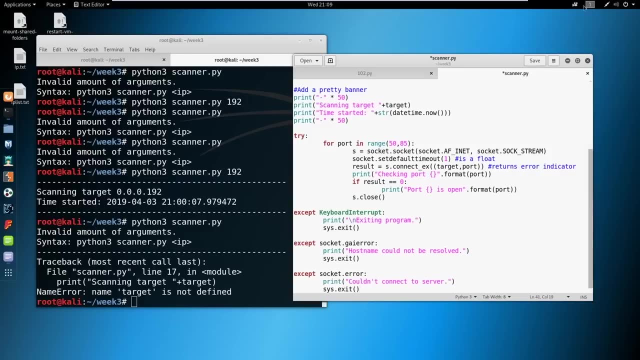 we'll just print: Couldn't connect to server and also sysexit: Okay, This is our shitty port scanner. There are lots of things wrong with this port scanner. This is a- I would say a- version one, When we're building something out. 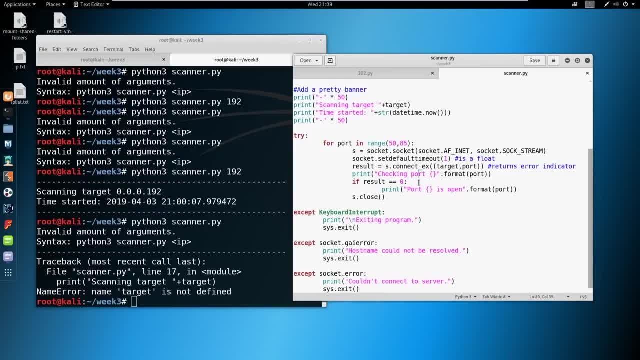 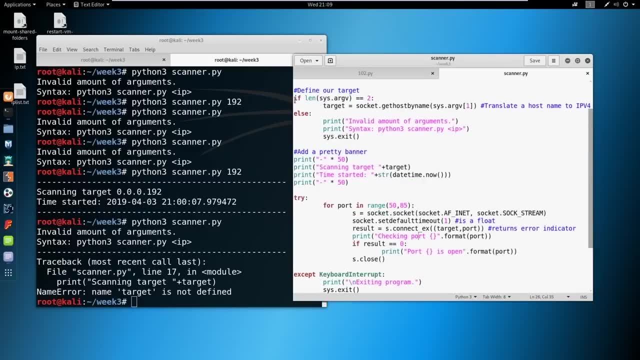 we come up with the concept, We say, okay, I know what I wanted to do And honestly it wouldn't even look this good. when we first do it right, We may come up with the okay, I know I wanted to find an argument. and if it doesn't work, 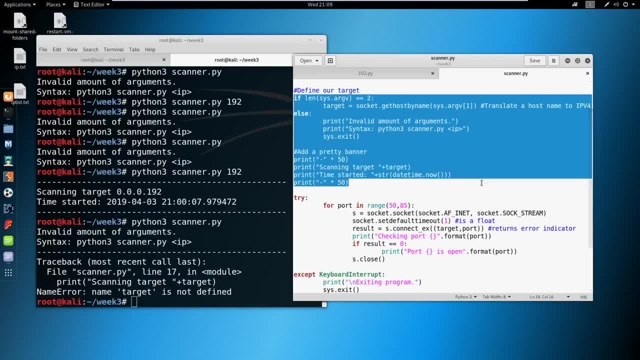 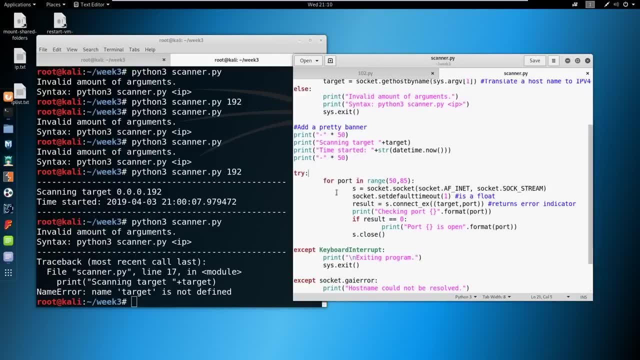 great, We'll add the pretty banner. That's pretty straightforward And we may not even put a try and we might just put a loop in right. We may even define a function or something else that works for this, instead of putting this try statement in. 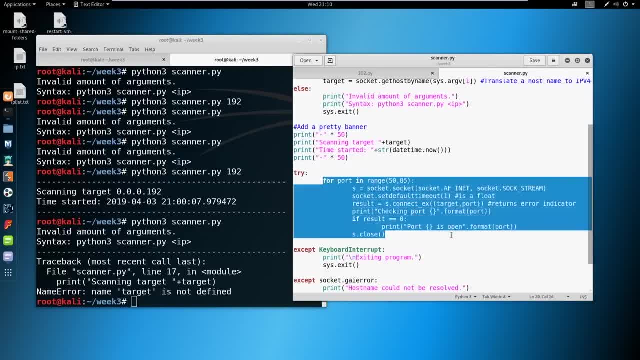 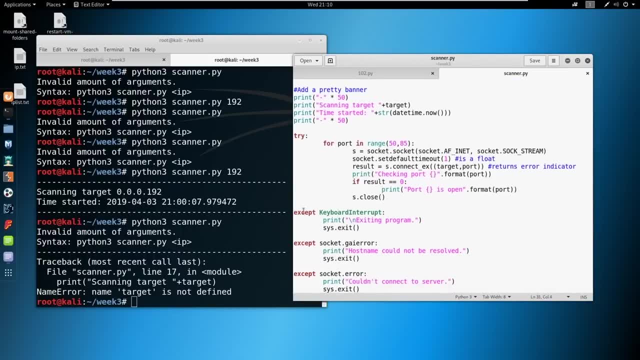 But we could loop through this range and try the connection, like we did here, And then we kind of have to figure out, figure out the exceptions as we go, Like we might try to hit control C for stuck and realize, ah crap. 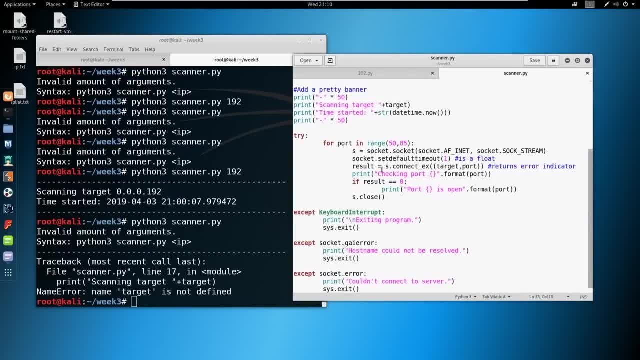 I didn't put a keyboard interrupt, So now I'm stuck right. Um, we would actually, if we were hitting control C without this keyboard interrupt, we would cancel the one loop and move on to the next loop. So you probably figured that out and you would probably have an instance where 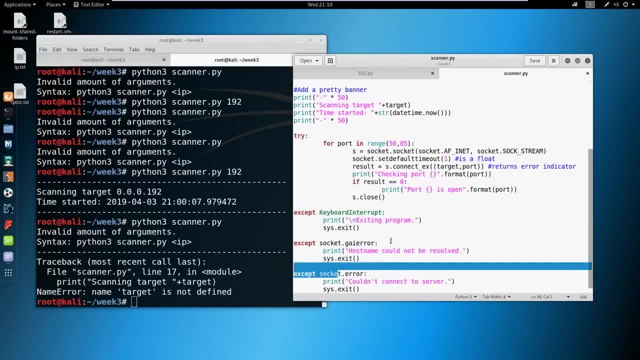 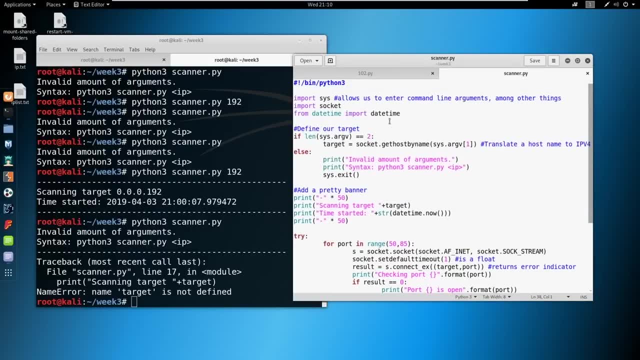 the host name isn't resolved and it gets stuck or hung up. Same thing with the socket error. So it's all trial and error. And now we look at this and we say, okay, well, we could probably improve this again. We talked about putting arg parse in here, so that if we wanted to declare specific ports, 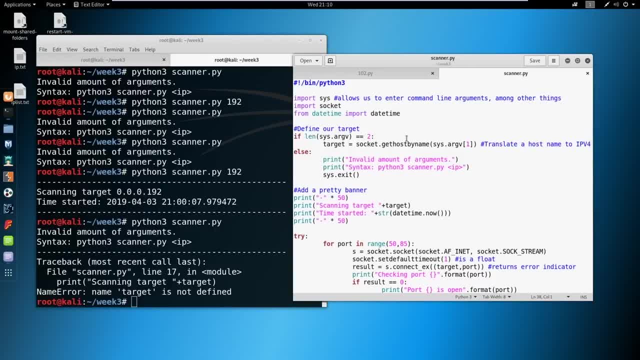 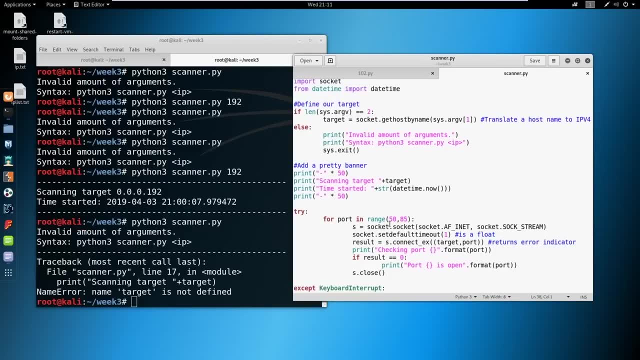 we can do that, And if we didn't declare ports, then we can run through top 1000, um, or all of them if we wanted to, depending on- uh, you know what we wanted to do. So something to think about, logically moving forward. 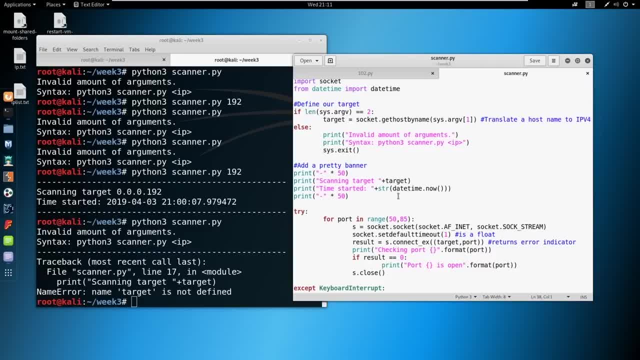 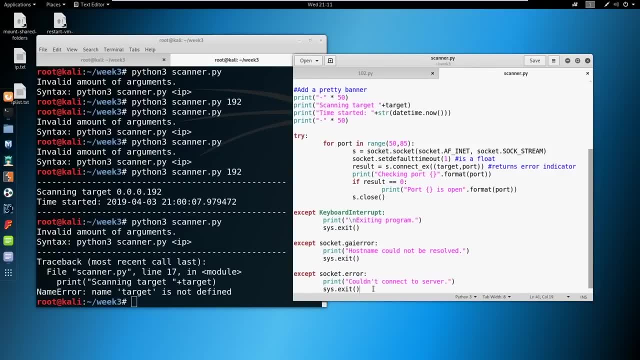 Another thing that we're not doing here is that we are- um, we're not threading. It is sockets dot GAI error. Sorry, let me put this down. I know I scrolled up. uh, no capital on the G, though, and not sockets. 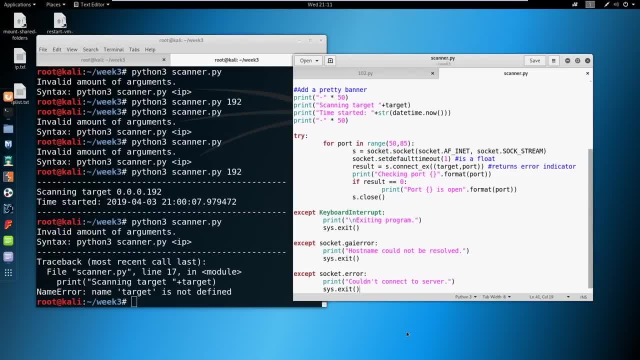 just socket all lowercase. So we need to do threading if we wanted to make this efficient, or else this is going to be slow as hell And this is why we're calling it a shitty port scanner. Um, we're going to run it. 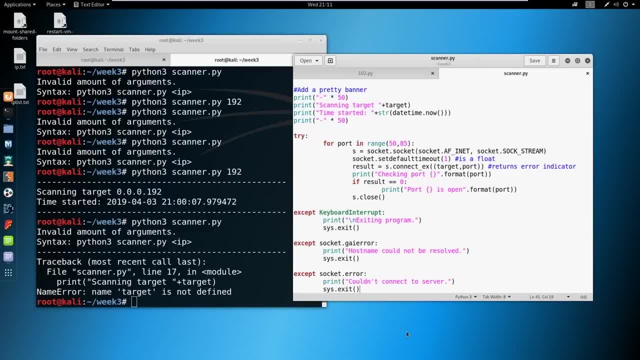 It may hang for a while before it even runs. Uh, if we do threading, then we'd be able to run multi processing right And allow it to actually uh, do its thing and execute quickly. Um, but we're not at that level of threading. 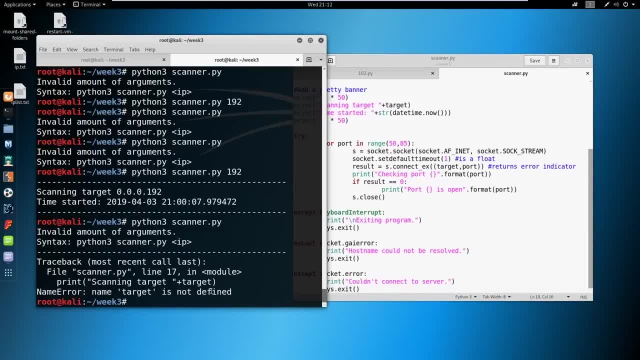 So we're going to build this little port scanner, like we just did, and we're going to try to run it. So go ahead and run it against your router or whatever you want. I'm running it against my router. Um, you may find no ports. 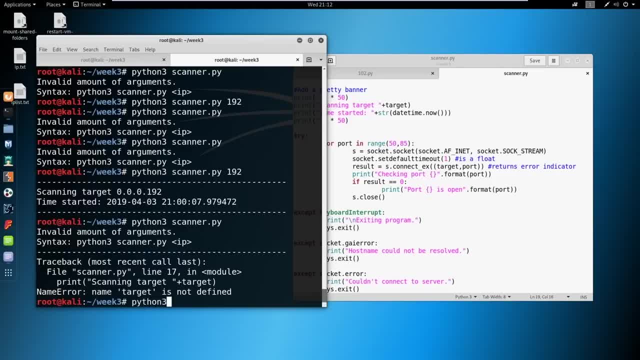 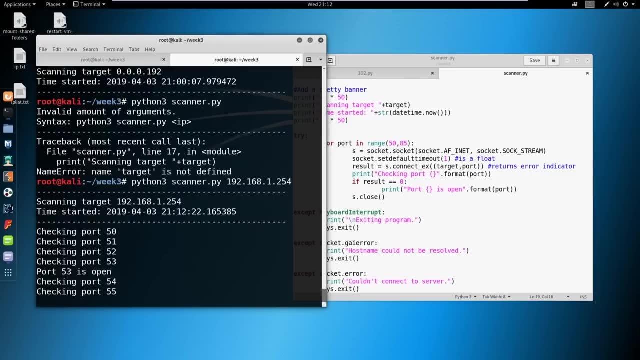 you may find some ports. So I'm going to say python3scannerpy And my router is at 192.168.1.254.. And you can see it's going through. port 53 is open. My router is checking for DNS. 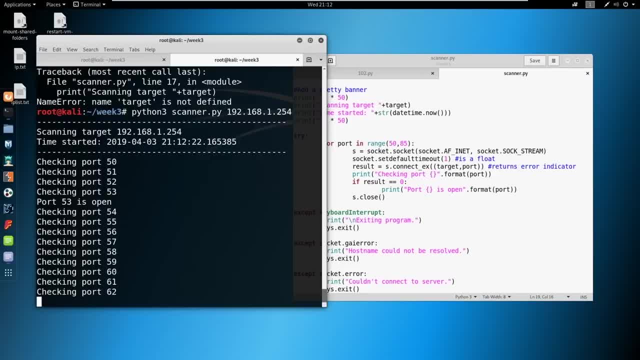 Or my router is doing DNS. It's not risky. I'm got DNS running. Heist 2000 is risky, Don't do it. All right, Port 80 should be open. I have a web interface. There we go. 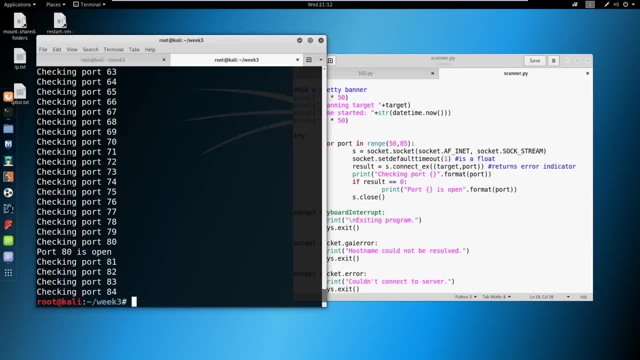 So you see how slow. this is right. This would take forever, Um, but if we do threading, we can run all these processes at once, or as many as possible that we could run at once. So just food for thought, And that is it. 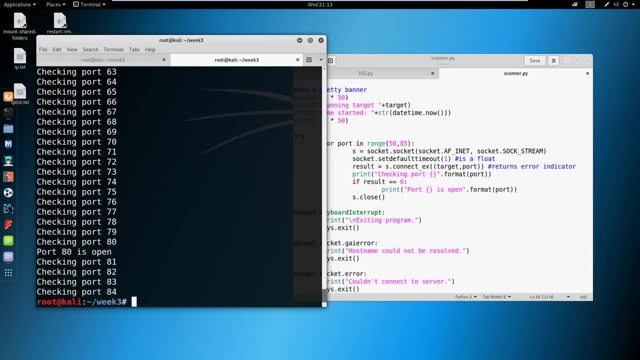 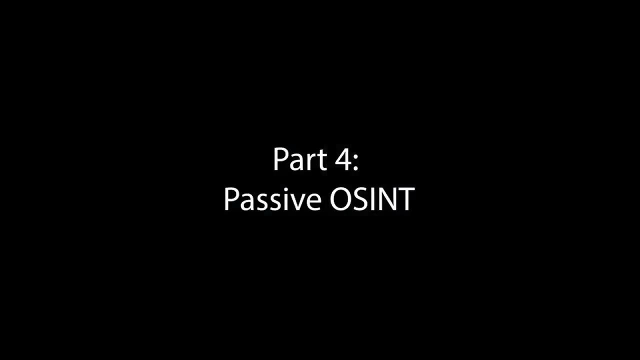 We are, we are done. This is faster than your end map. I don't think it's faster than your end map. Your end map is doing a lot more than just checking if a port's open, Usually the top 1000 and map scan. that runs fast. 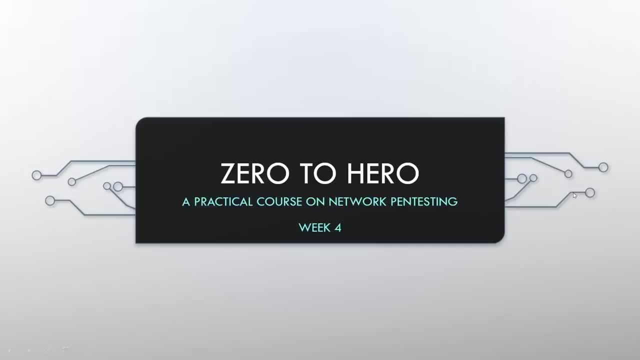 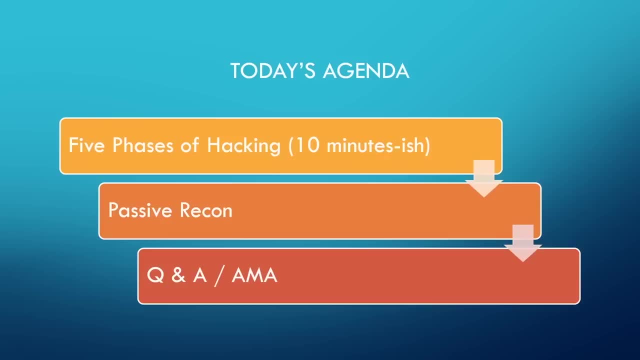 So welcome to week four. We are covering the five phases of hacking. maybe 10 minutes, probably five minutes. It won't take that long. Uh, then we're going to talk about passive recon or OSINT, and then we'll do the Q and a AMA, like we always do. 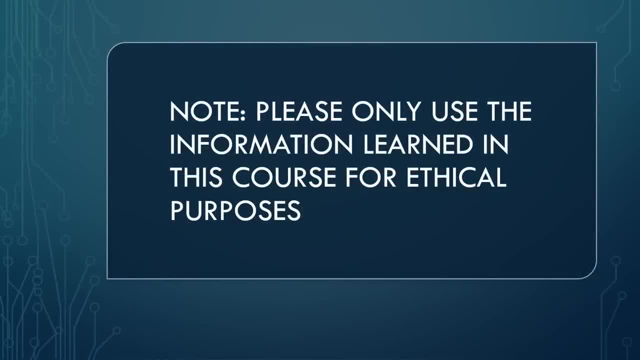 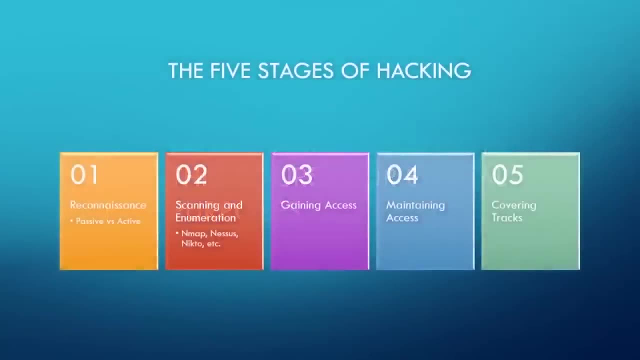 Okay, Note: please only use the information learned in this course for ethical purposes. From here on out, we are getting into the hacking phase of the course. So please, please, stay ethical. Don't. don't join the dark side. This is dark enough. with that being said, 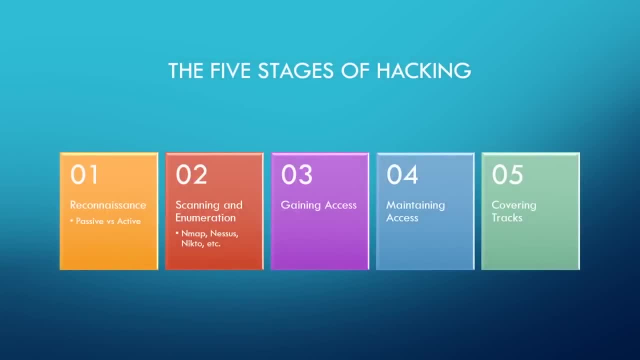 let's go ahead and cover the five stages of hacking. So stage one is reconnaissance. Now, reconnaissance is basically information gathering. So we have passive and we have active. I would actually consider active to be more of a level two or a scanning phase. 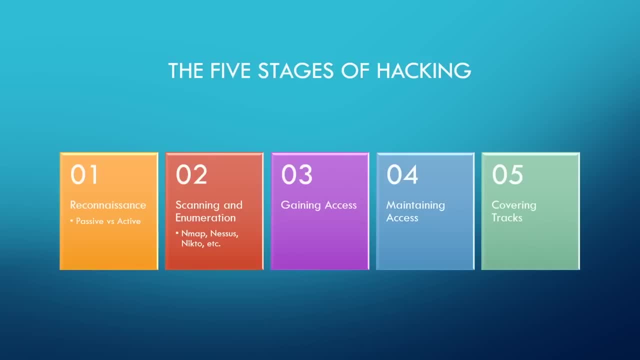 Passive is when we do information gathering that doesn't involve the client or the entity itself, right? So we're going to be looking up maybe LinkedIn information or Google information, Twitter, Facebook, whatever we can to gather information, but we're not going to be. 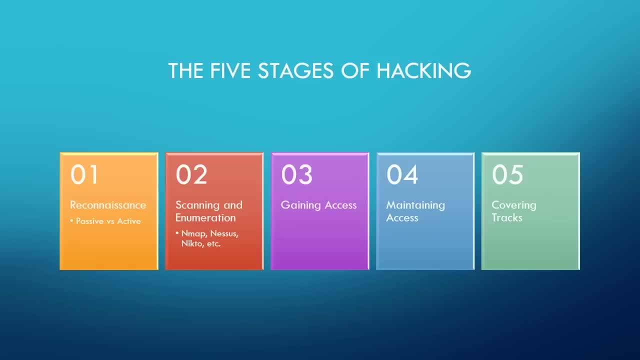 um, attempting any scans on that server or scans against the host, um, et cetera. That's more of active reconnaissance And I consider that to actually be scanning Um. so once we gather the information that we need- and we're going to be talking about phase one right now- 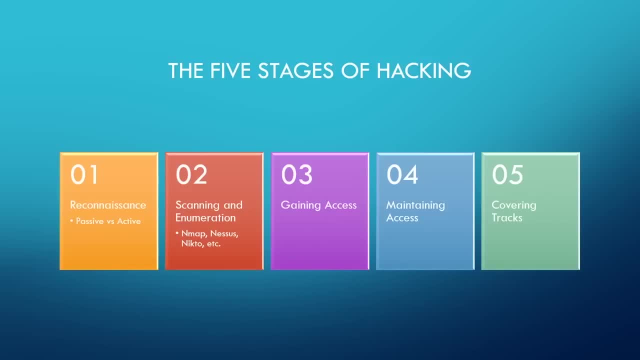 and as we go through the course, we're going to hit hard on phases two and three. we will touch on four and five as well. Uh, but as a pen tester, you don't need four and five as much. I'm not saying that they're not important. 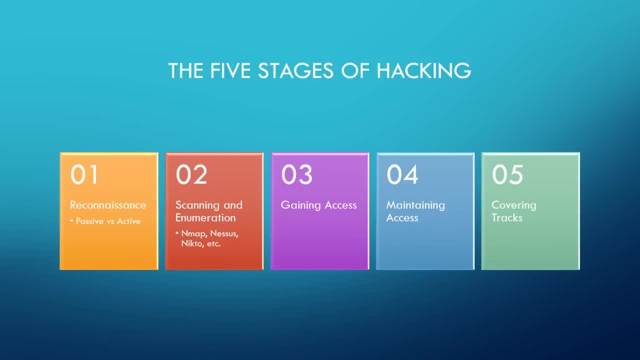 but we'll talk about um, how you would maintain access if you need to, and how to clean up when you're done with a pen test. Now, if you're doing red teaming, uh, it becomes a little different in four and five become more important. 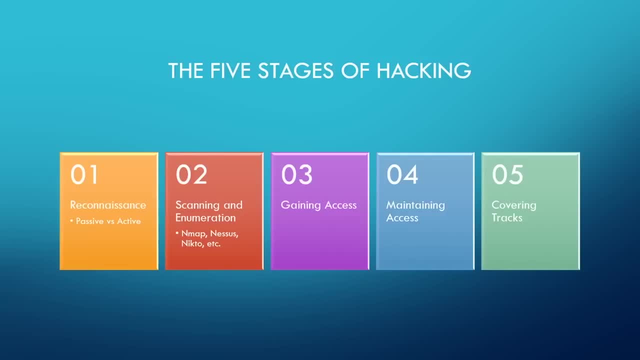 Um, if you're acting like you're a APT or something like that. So once we do phase one, we're going to go ahead and go into phase two, which is scanning and enumeration. This is your M app, your Nessus. 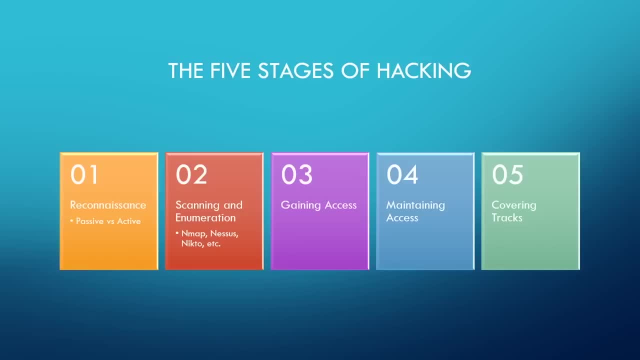 your Nikto, um, your Metasploit can do scanning. Open boss is a scanner. So we'll cover some of the different scanning tools, how to read those, what ports to cover, you know, et cetera, As we get into that. 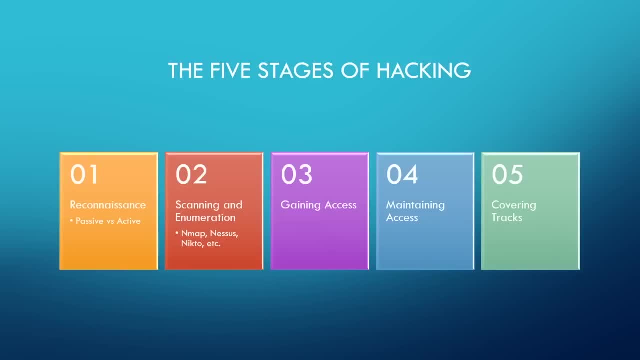 I won't dive too much into that right now. Um, and then gaining access. So once we do our scanning enumeration, steps one and steps to really step two- I would consider probably the most important, but the more information and the more. 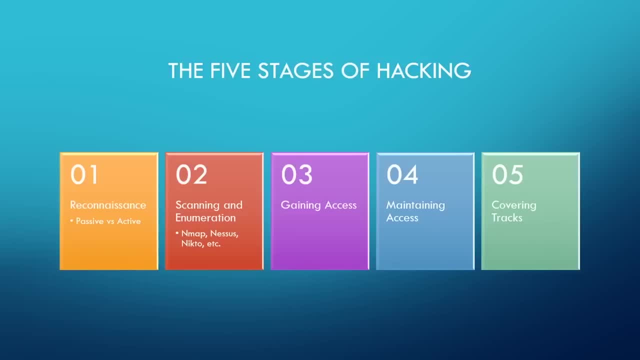 uh, you know, the more enumeration you do, the better off you are. So hacking is all enumeration. uh, enumeration, enumeration, enumeration. Even after you gain access, there's a whole nother level of enumeration, especially if you're just a low privilege user. 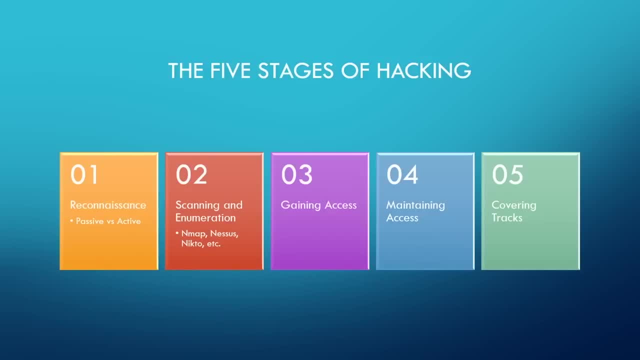 or even if you have a domain admin account, um doesn't mean you have the goods right Just because your domain admin there's still might be some information out there that you want or need and you need to figure out where that's at and find it. 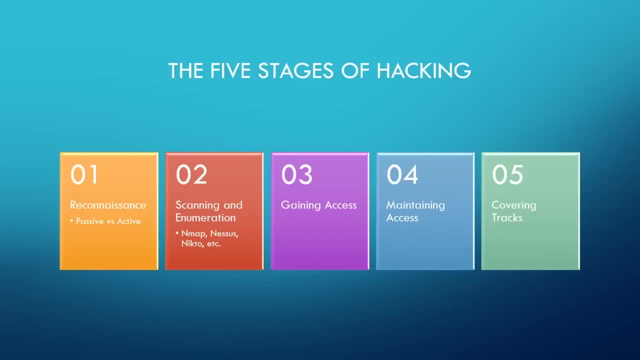 Uh, so we're going to play a big part here, or do a big part, in terms of learning how to scan properly and learning how to enumerate, Uh, but that will be later on in the course, but these are the most important lessons. 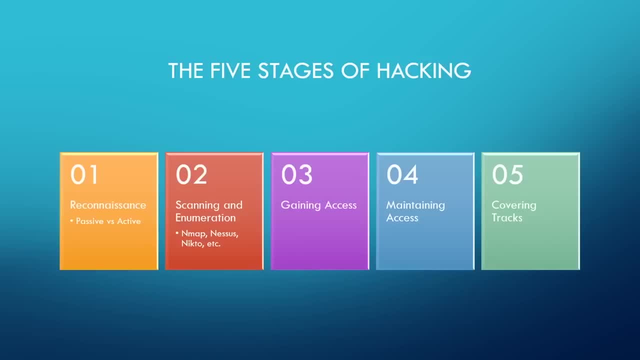 Um, I can show you how to exploit all day, but if you don't know how to find these things, uh, you, you're not going to be a good, good pen tester, good hacker, et cetera. Uh, 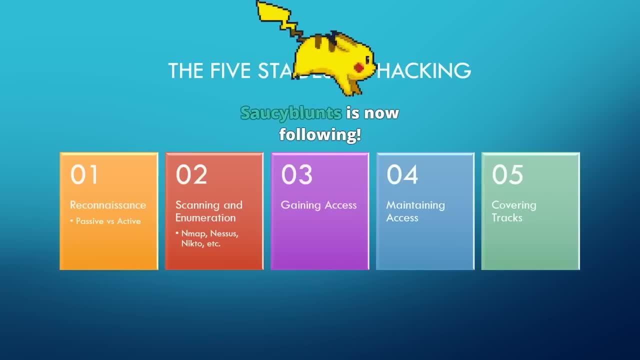 so once we do our scanning enumeration, we find a way in. this is called gaining access, Uh. so we gain access either through some sort of exploits, social engineering, uh, et cetera. Once we have access, we want to maintain access. 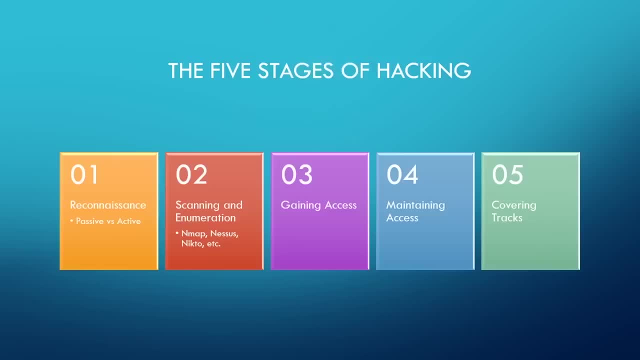 right. So we are uh looking for a way to uh maintain access in the network, not get detected, um, depending on how we want to do it, What if we have a session and, uh, you know, something happens where they reboot the machine and we lose the session? 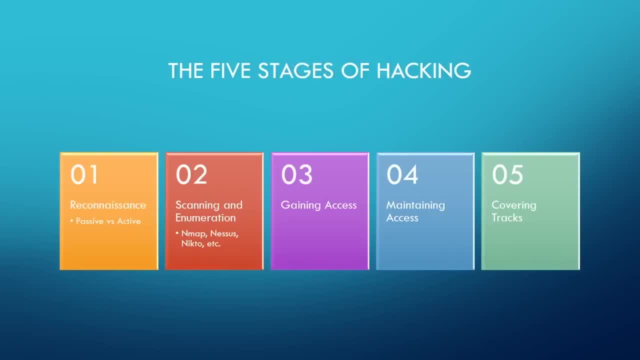 right, What? how can we prevent that? How can we be on um multiple- you know multiple interfaces and not get disconnected or detected? Uh, so we'll talk about that, and we'll talk about covering tracks as well, Um. 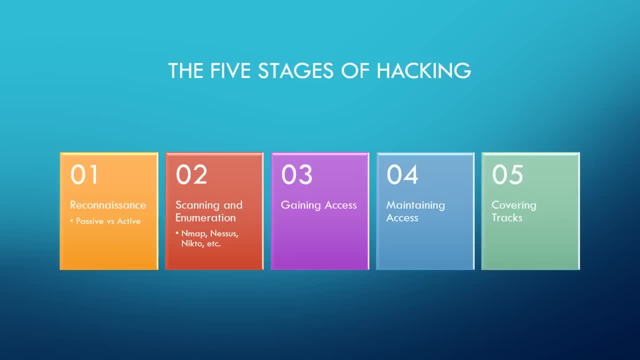 there's a lot of tools that we'll do that will auto cover our tracks, Uh. so that's really, uh, a lot of things that we'll do. So if we're in a shell, like, for example, you'll see me use P S exec. 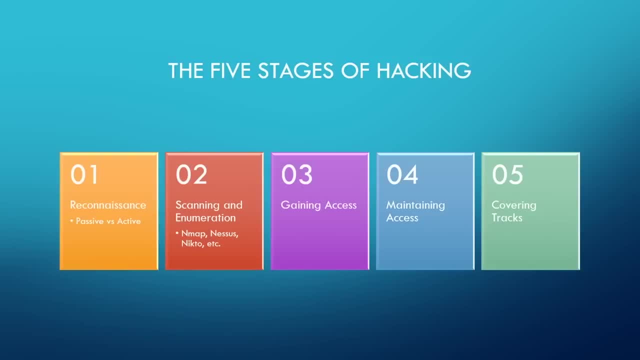 P S exec uses SMB credentials to get a shell. Uh, so when we're in there, what'll happen is you'll: you'll connect to the SMB server, It'll upload a reverse shell, It'll connect to the reverse shell and then it'll delete it for you. 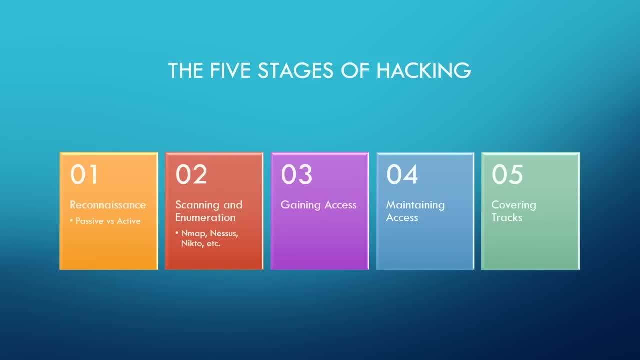 Um, so some programs do cover your tracks for you, but you don't want to leave malware behind or any information that you have uh been there behind. that includes, if you're uh, if you're pen testing really not important on that aspect. 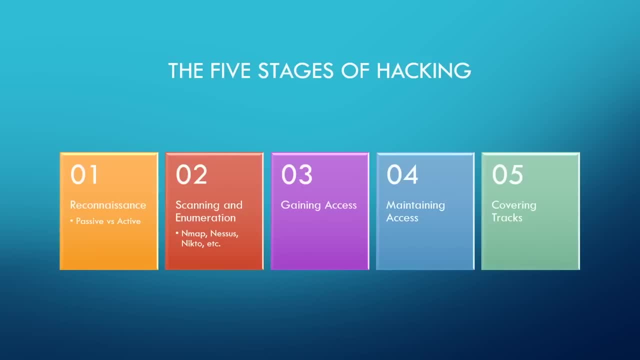 like deleting logs, But if you're uh running a program, uh an APT, you're definitely going to be trying to uh trying to cover your tracks. So, uh, thank you for the donation, Bammers. 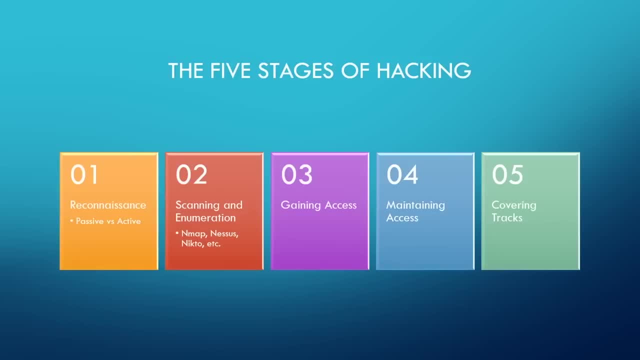 I appreciate that, Brent. uh $101.. That's a lot. Thank you so much. Um, and Rory says P S execs very loud. Don't be fooled. This is true, Uh, depends on who you're going up against. 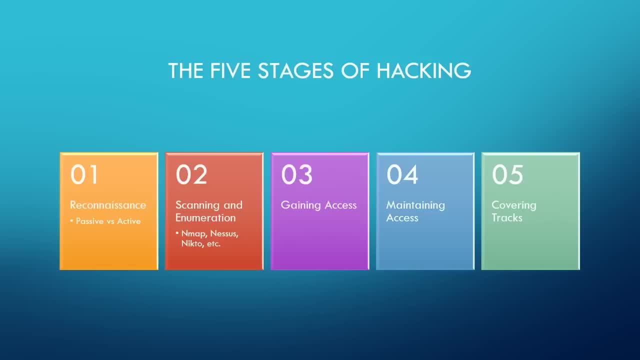 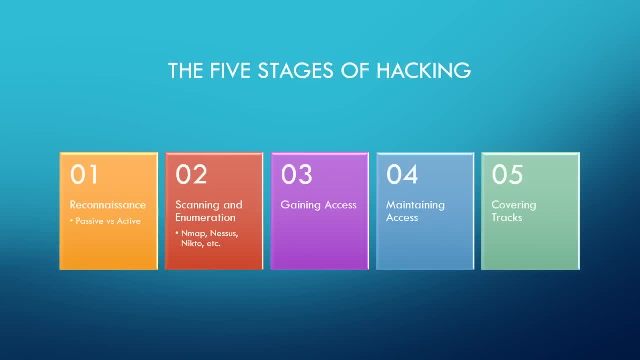 either have their- uh, their SIM tuned correctly or they're not running a SIM at all. So that's really it. It's. it's more of a cyclical cycle, Right Um you? sometimes when you view this chart. 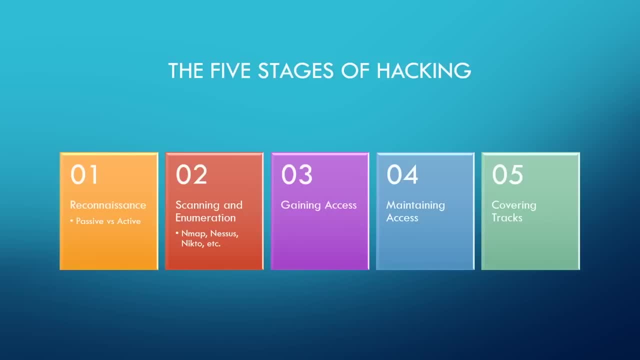 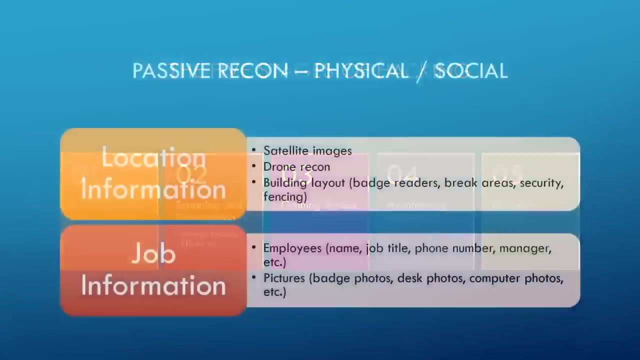 you see it in a One to five, in a circle, Um, but you, you go through these steps, uh, doing any sort of hacking. So it's important that we go in order and then talk about these things. So today we're going to be talking about passive recon And I'm breaking it down. 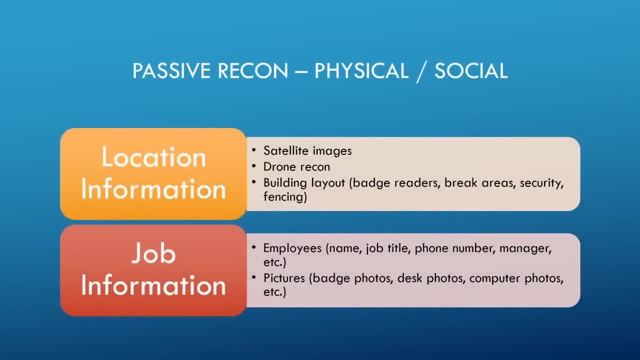 into a couple different types here And I'm not going to do death by PowerPoint the whole time. Basically, what I want to talk about is: let's talk about physical and social first. So if I'm doing recon for physical or social, some things I might want to look at, So maybe 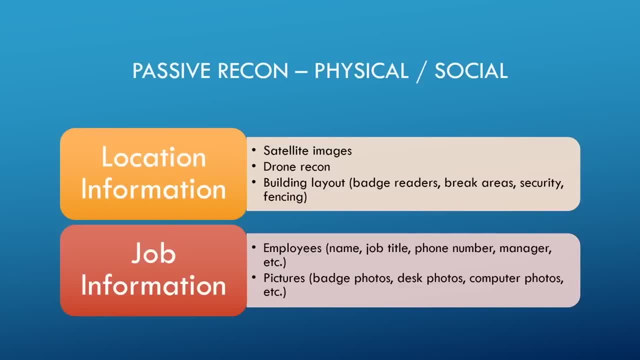 satellite images, right? Or I have a coworker who does great physical work and he actually has a drone that he flies out and around the building to look at the building layout, And that's another thing, right, Building layout. So with these, you want to know where the badge readers are. 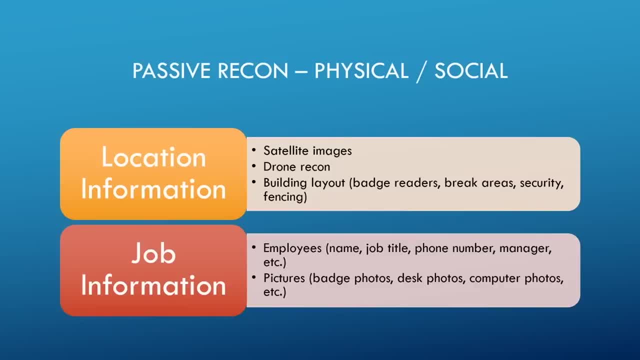 where the break areas are, what the security looks like, what type of fencing there is, Are people leaving Doors open. You know what kind of information can you get about the location. So you want to know what areas you might want to hit hard and where to attack the weak points. So you know. 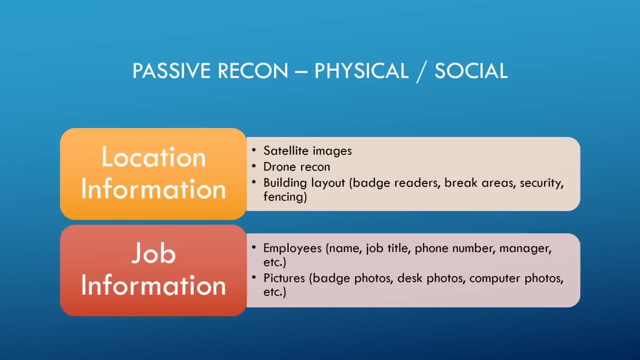 you're probably not going through the front door. Sometimes you have to go through the front door when you're doing a physical, But a lot of times you don't have to do that at all. There's a lot of sneakier ways: cloning badges, a lot of things you could do, Social engineering, you know, go by. 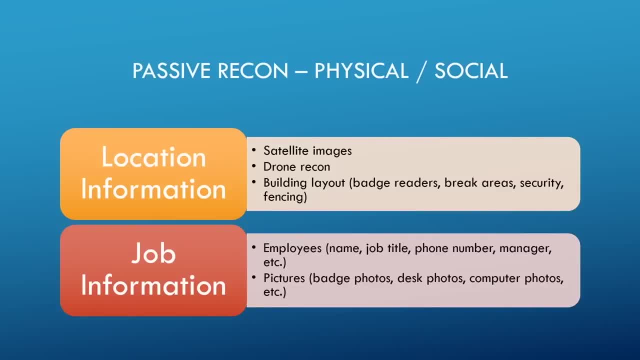 the smoke area And chat somebody up and then just have them hold the door for you. You know tailgating everything. You want to know your building layout and location information as best as possible, Also going into a social aspect in these both. this starts to become important for not just 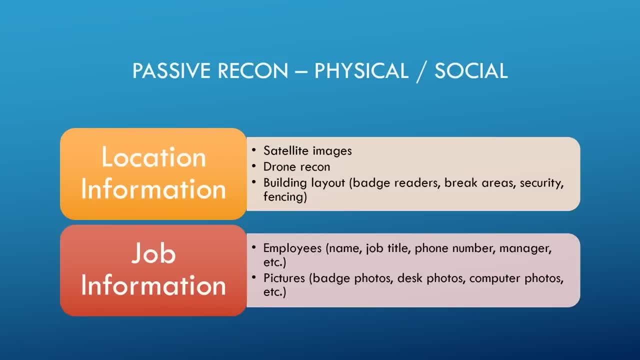 physical, but when you're starting to do host assessments and web assessments as well. So we're interested in job information, right, Like who the employees are, what's their name, what's their job title, what's their phone number, who's their manager You want to try to build out. 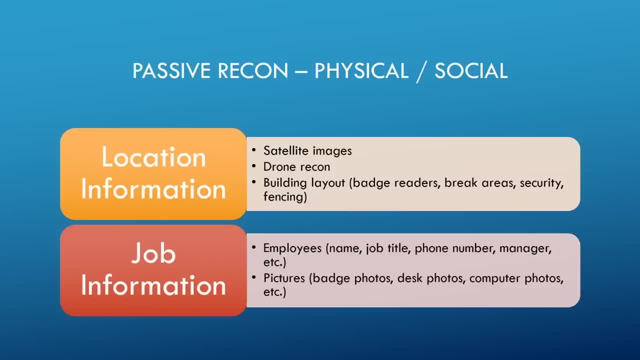 some sort of you know, I guess- topology for employees. You got to figure out who you're going to target, Like today, I was doing a debrief on a client that we had and they had on the public web their help desk portal. but their help desk portal listed every single name of their help desk. 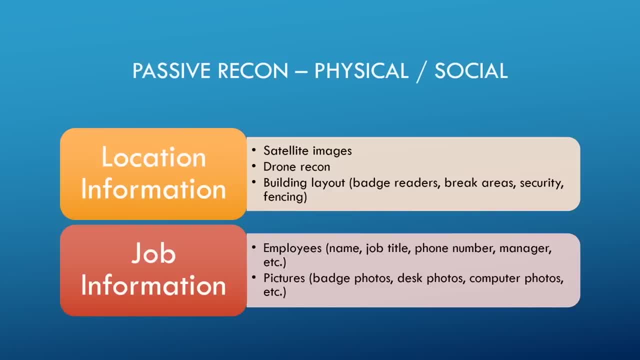 employees, and there's about 10 of them, That's just. you know. it's not an exploit, but that's really good information for me If I want to call another employee and say: hey, I'm Joe from help desk, you know, and Robert's my manager. 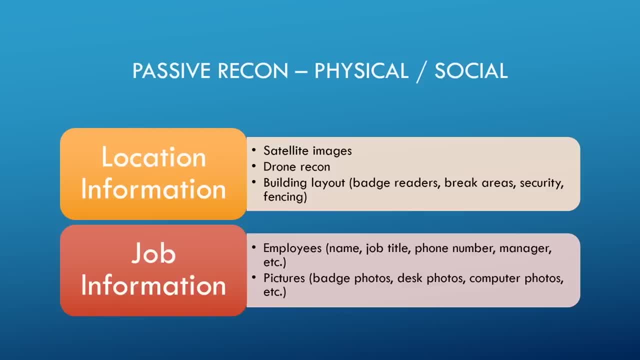 whoever, and you try to impersonate somebody. So as much information as you can gather and what field they're in, what they do, you want to try to map out as much as possible. You should know who the VPs are, who the CEO is, et cetera. You don't want to, you know, say the wrong name. 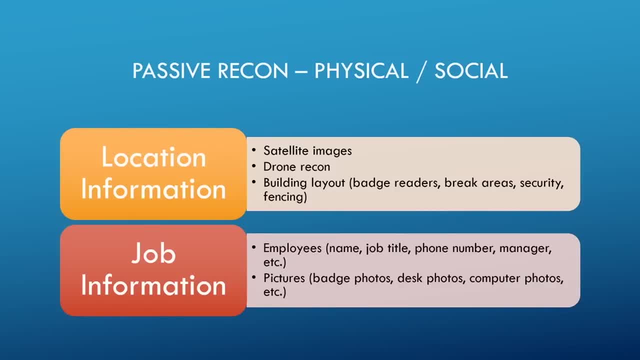 to the wrong person and ruin everything, especially if you're on a physical level Or a social engineering engagement. That also includes pictures. So one thing that we look for when we're doing physical engagements is: we'll find who the employees are, and then we'll look. 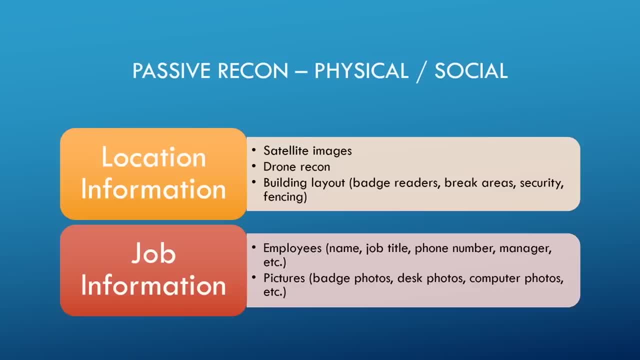 them up on Twitter, We'll look them up on Facebook, We'll look them up on LinkedIn And you will not believe how many times they have their badge in a picture, their desk in a picture, computer photos. I mean there's so much information that we can find. If you've got a badge photo, okay, we know. 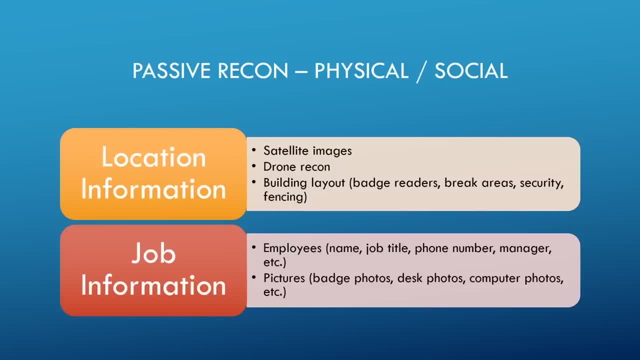 image of your badge. right? If you've got a desk photo, what are we looking at? Well, we can be able to see what the letterhead is, Perhaps if you've got some letterhead on your desk or like a company calendar. we're just trying to look for logos, design, anything that we can use to make a fake. 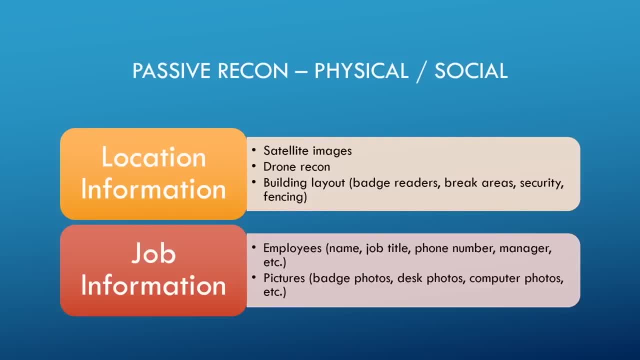 badge, if we need to, You know. and computer photos. I've come across plenty of computer photos that show what kind of software you're running. You're going to tell me what, maybe what kind of outlook if you're using. you know, like I've seen some. you know, I've seen some. 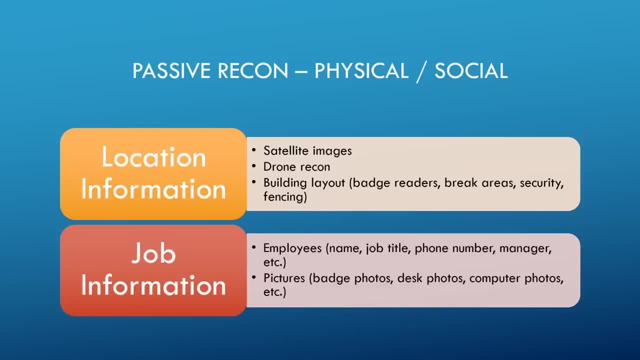 Slack, channels, information, a lot of things that people don't think about. right Like I've seen accounting information on a photo posted on Twitter before because somebody took a photo of their desk. People are the weakest link. They'll always be the weakest link You could have. the 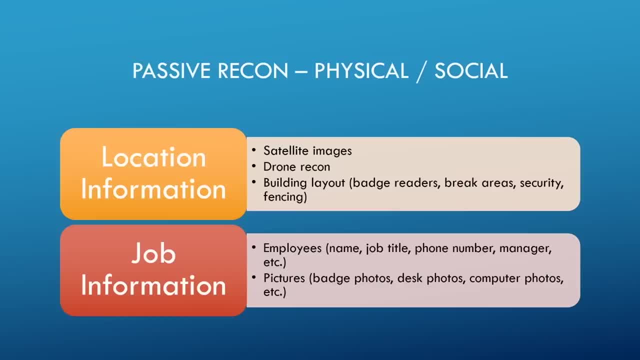 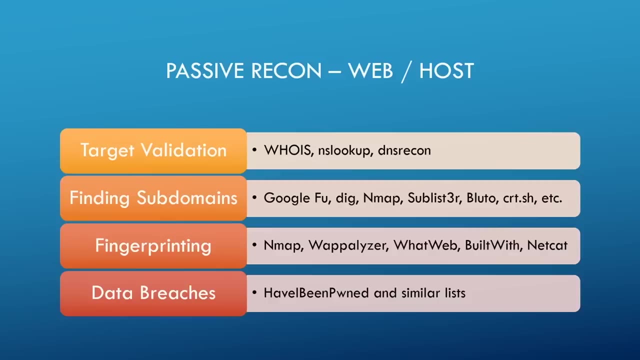 strongest barriers possible and it won't matter, right? I mean? so a lot of this is employee training and et cetera, but this is the kind of information that we are after, And a lot of people are talking about badge cloning, So we use a tool. it was about two. 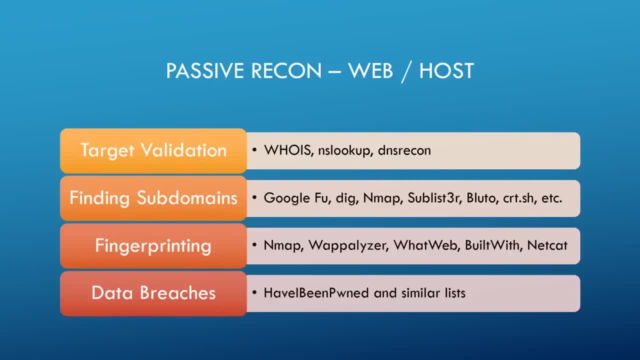 grand It's called. it's called Boss Cloner. Basically, you can build it yourself for about 500 bucks. It gives you all the instructions, but if you want it built for you, it's two grand. It doesn't work with every type of RFID, but if you get close enough you can pretty much capture. 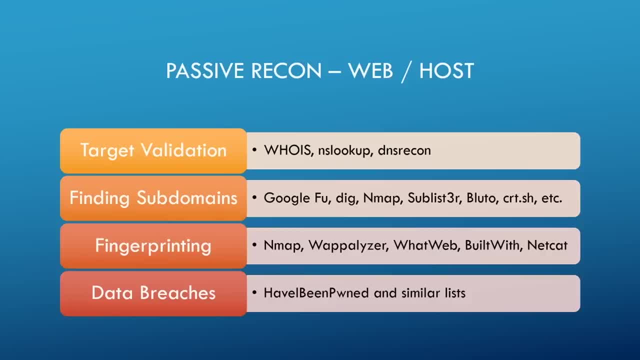 RFID and then use that to gain entry. So it's very, very easy. We're not going to go into to the physical side of things and how to you know hack doors and all that stuff. I have a really good co-worker. 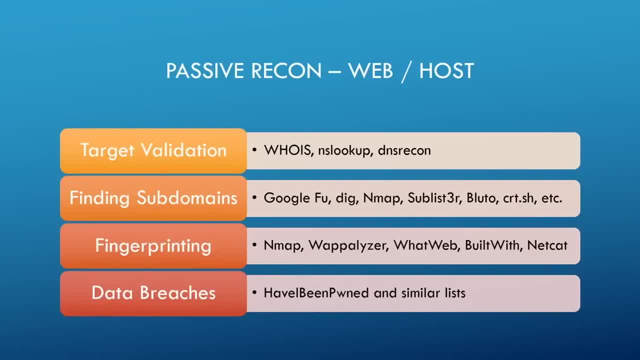 who I would love to bring in for that And maybe I will get him to bring in. He is by far the best physical pen tester I've come across. So if we do a physical lesson later on down the road, I think I would, I would definitely bring him in. So when we come across- so let's say the passive recon, 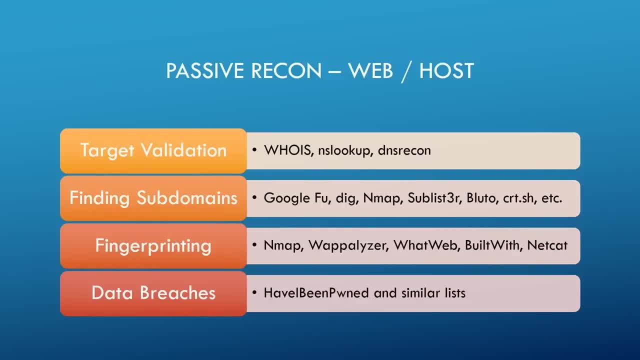 for the web and the host. well, we need to do a couple of things as well. So we need to do a couple of things as well. So we got to do target validation right. We can do that with who is NS lookup, DNS recon? There's a ton of tools. Basically, we need to verify that the IP space. 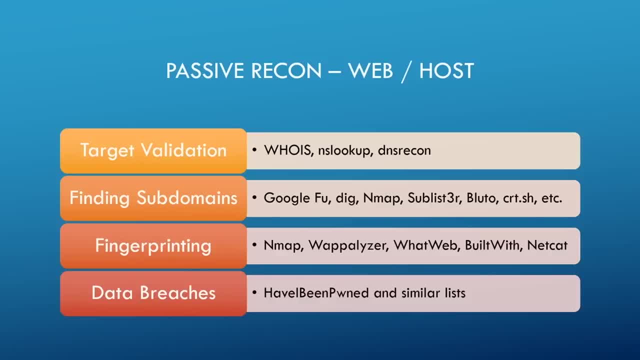 or the host or whatever they give us is indeed their ownership. A lot of times you're going to get a subnet or, uh, you know, just a IP range, and they'll include the router for the ISP in there or something like that. That's not theirs, Doesn't belong to them, So we're going to have to. 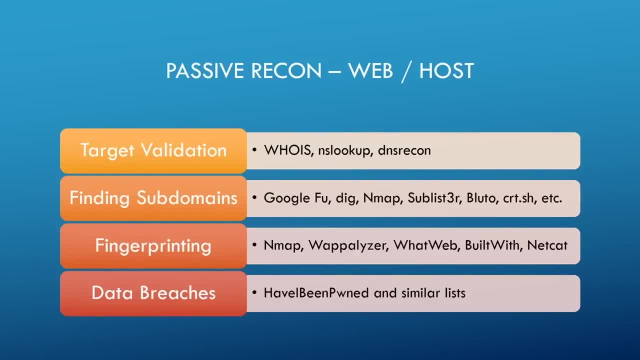 and you shouldn't be scanning or pen testing against it. Uh, so it's important that you look up the website that they give you and make sure that they own it, um, that they didn't make a typo or any sort of information like that. So, um, but also for recon terms, um, who is is useful. 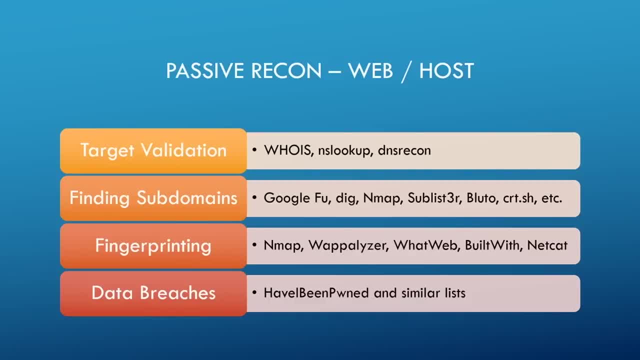 Sometimes they don't put, uh, they don't put a protected, I guess, owner in there, They'll put their own owner. Sometimes it's not private, Uh, so you might be able to get um owner information with a address, et cetera. Mostly everybody goes the private route, Uh, but some people don't uh. 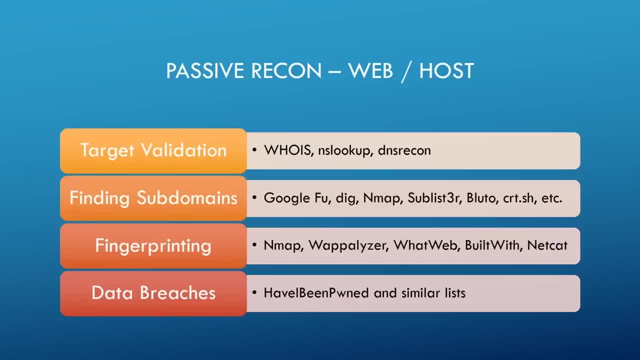 NS lookup, DNS recon- Uh, we use these tools for a lot of things. Uh, finding subdomains is important as well. Uh, so you could just do some Google foo. We could use dig and map sublister Bluto. 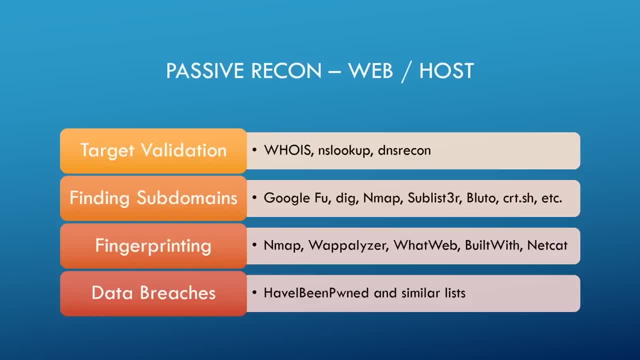 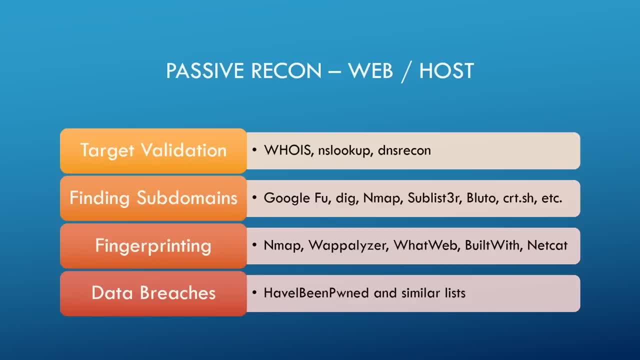 uh, just to find a little bit more information about the site. maybe we'll find something like a devgooglecom or something along those lines. Um, you know, like whatever site we're looking for, maybe they have a dev environment where they didn't want us to know about. Um, and we'll find. 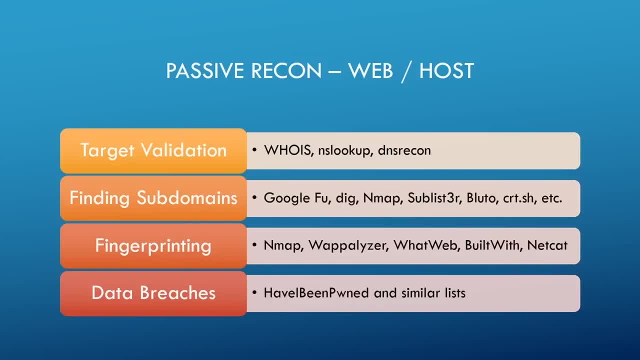 that information online. Uh, same thing with fingerprinting, and fingerprinting I'm I'm kind of iffy on because I kind of call it active recon because you're going to the website itself, uh, with a lot of this. So end map. it's definitely active recon because we're going to scan against. 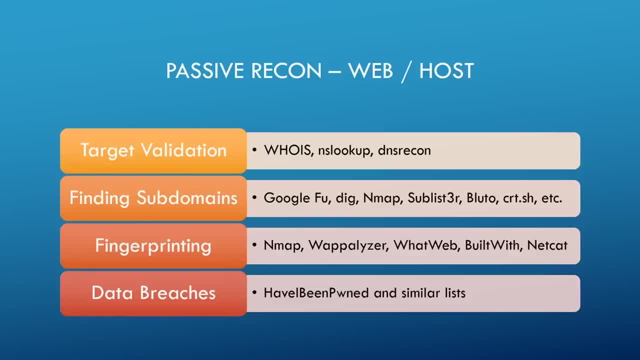 it. Wapalizer is a tool that we use to see what they're running. Basically, with fingerprinting, we're trying to see, um, what type of tools or backend that that website or host is using. Typically, this is for a website, Um, but we want to know, you know, what type of 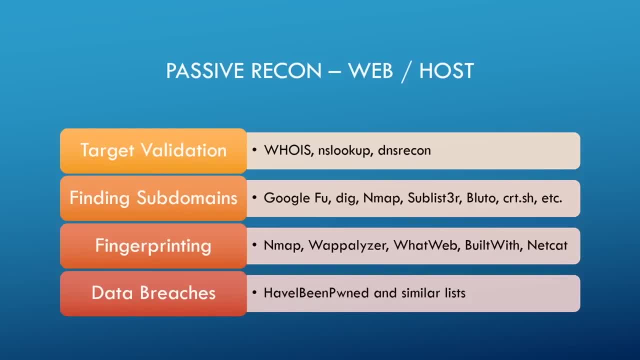 of software might be running. So what web is good for that? built with is good for that. Even using netcat to get the headers of the site might tell you some information. Uh, so being able to fingerprint a host, uh, it falls under passive slash. active, I would call. 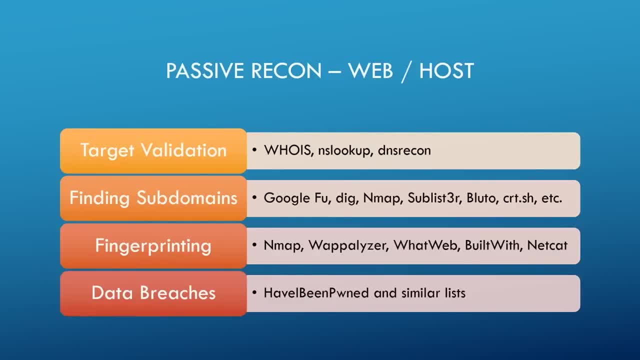 it. You can do a little bit of both, So it depends on what you do to make it passive or active here. And then, lastly, data breaches. So have I been pwned, or similar list? Uh, so tools that we've. 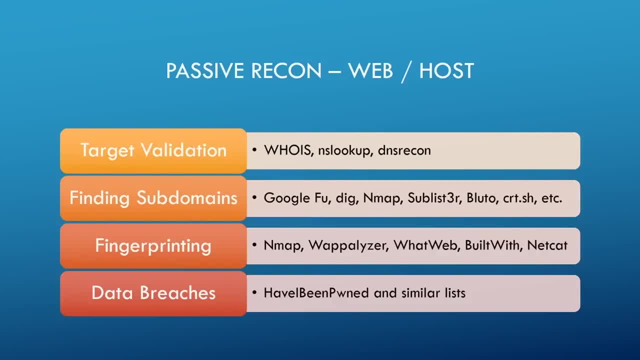 covered here, um, like Bluto itself or the harvester. uh, some of these will check through. I don't know if the harvester does. actually, some of these will check through lists to see, um, if there have been credentials found for. 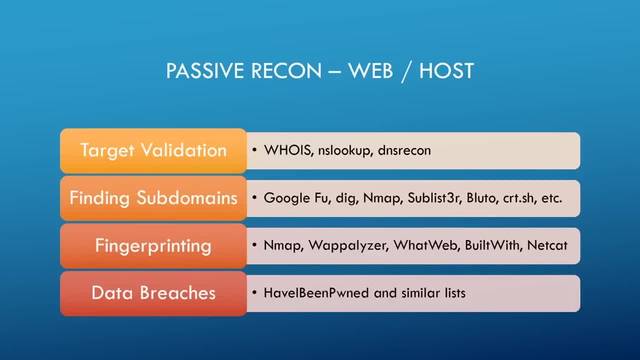 that domain in. have I been pwned? Uh, but we're going to talk about this a little bit heavy here And then in a later lesson we get into hacking. Um, so tonight I'm going to show you a script that I wrote in bash, And what we'll do is basically what it does is run through a. 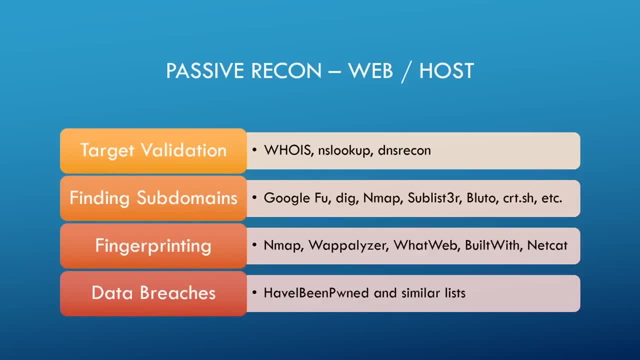 clear text, password list or try to find passwords. Uh, you know, through for a domain that we supply. So we'll see how that works and how we can use it and think about how we can use it. Um, so, plenty more tools than what I noted here And we'll cover. 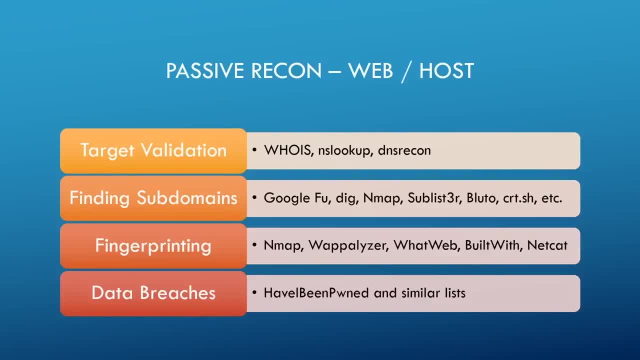 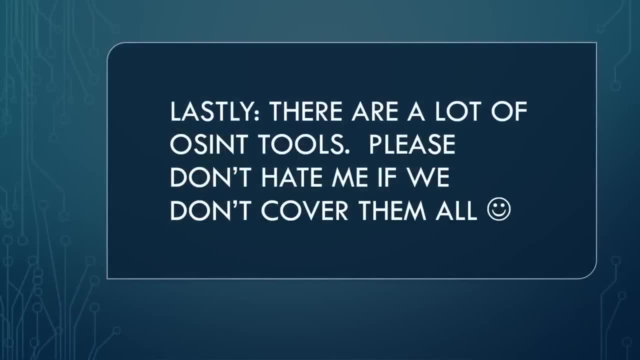 some of these we'll cover, not all of these, and we'll- uh, we'll just go as we go. So, lastly, before we get started, like I just said, there are a lot of OSINT tools. Please don't hate me. 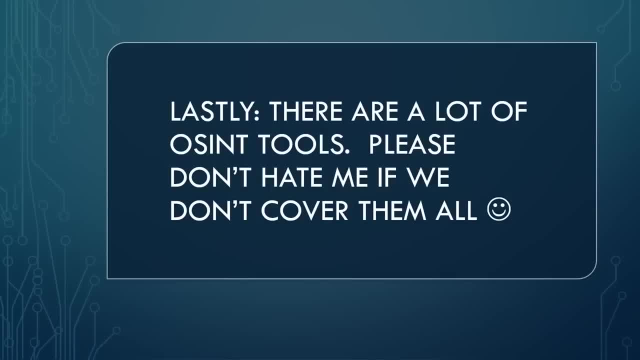 if we don't cover them all. I know you guys know a ton about OSINT tools, I'm sure, Um, but we're not going to be able to get to all of them, So I'm going to show you a little bit. 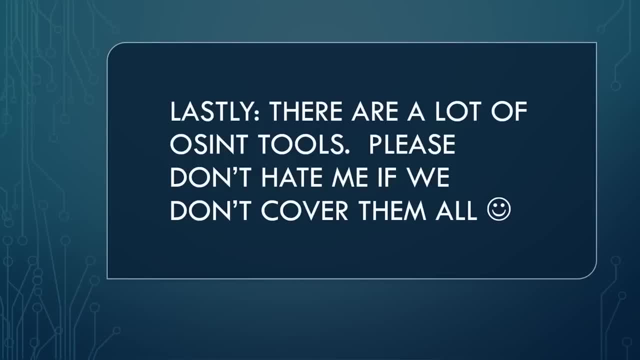 I don't even know half of them. Probably There's so many cool little things out there that um are, I'm sure, are helpful. but what I'm going to do is I'm going to show you what I know, how I would do it on an assessment And what we're actually going to do tonight. 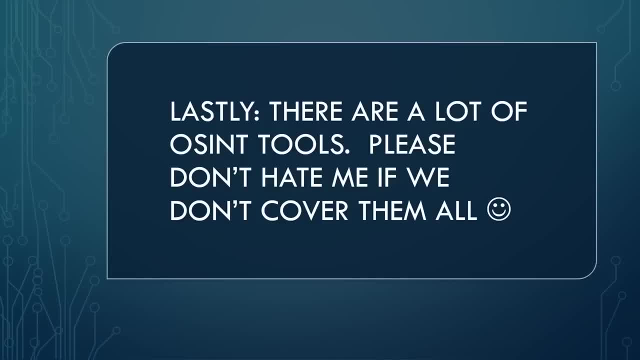 is: we are going to go through, um, we're going to go through, uh, a, a client of our choice. Basically, what I'm going to do is I'm going to go to bug crowd. We're going to pick out some. 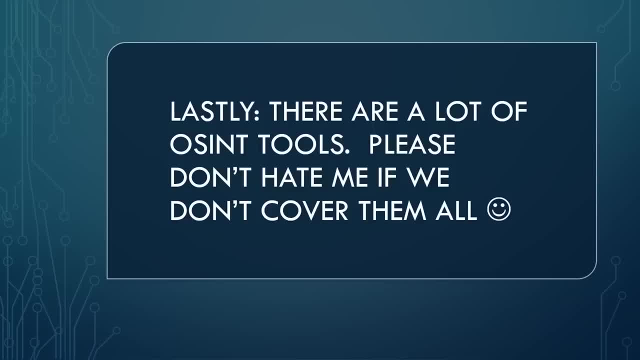 clients that might interest us. What I want to do is I want to pick something that may be um, medium to smaller size. I don't want like a large client cause that's just going to take too long to dig through. I want something that we can. 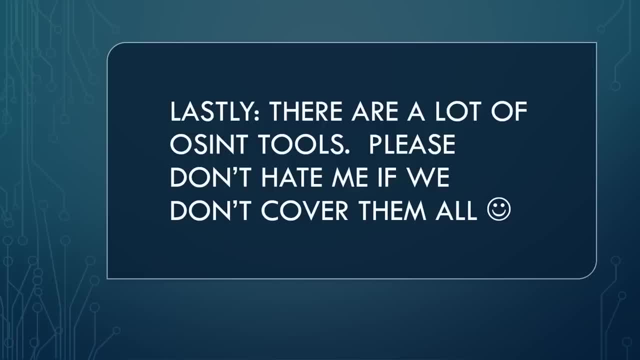 gather a lot of information on in a short period of time. Um, so we'll throw out some, some names or companies, and then we'll uh try to do OSINT on them. Uh, no, you can't pick me, but you're. 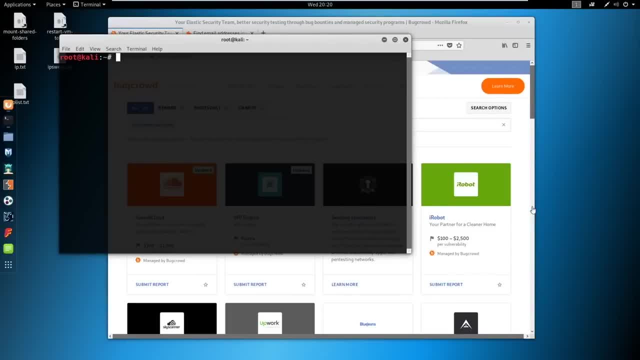 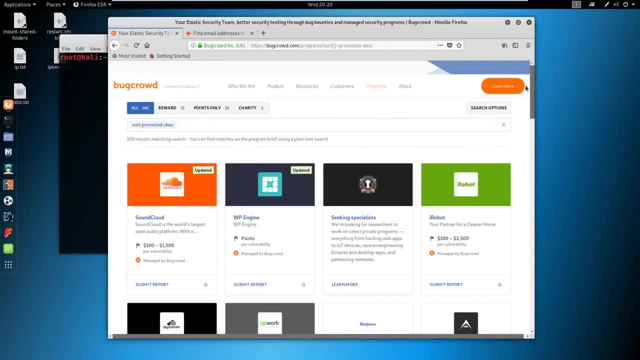 welcome to OSINT me. You guys have already been doing that today, So you're- uh, you're welcome to continue doing that, But the goal here today, too, is we're going to do this collectively, as a group. I'm going to show you some of the things. 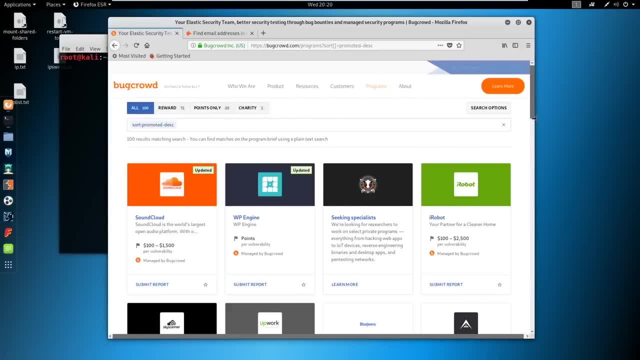 that we can look for and that we can do, but at the same time I want you guys to be looking on your own and then posting some information in the chat. Uh, that way we, we have that information and we can kind of collectively do this as a group. Um, so what we're going to do is, if you 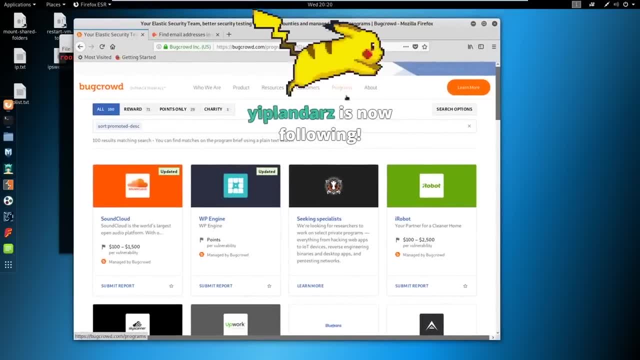 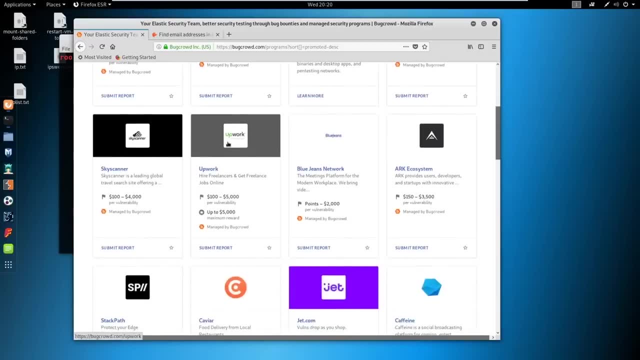 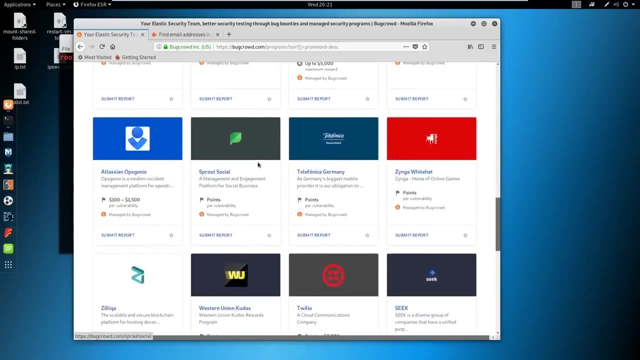 go to bug crowdcom and you do the programs. if you do programs up here, uh, basically, what we're going to do is we're going to pick one out of here that we want to do. Um, so I would pick something on the smaller side if we had that choice. So, but we can pick. 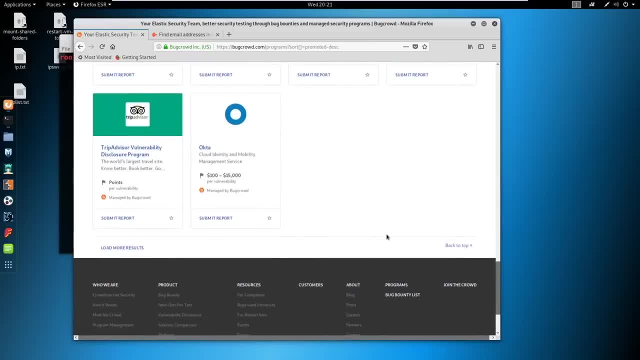 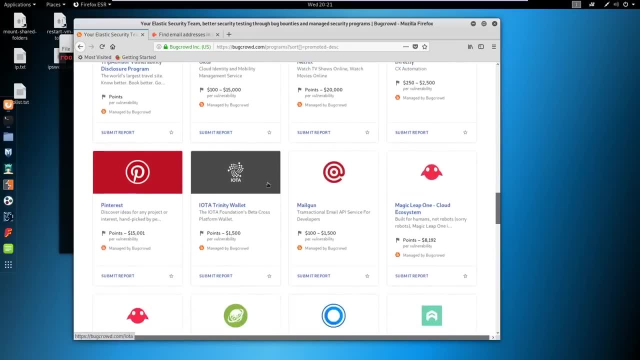 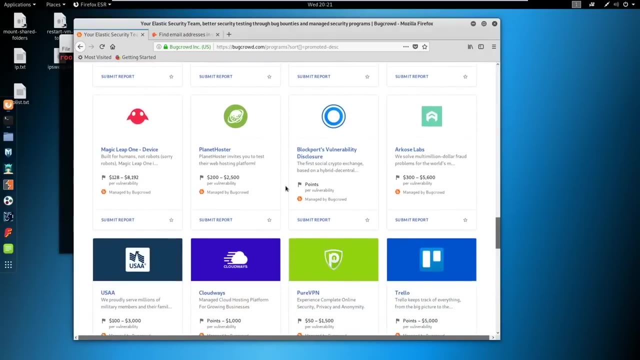 um, something on the medium to medium to smaller size, if we can. So if you see anything in here that is of interest, we can do it. Or what we can do is- I was messing around with Tesla before- per uh, Davey's recommendation. Actually, we can do Tesla. 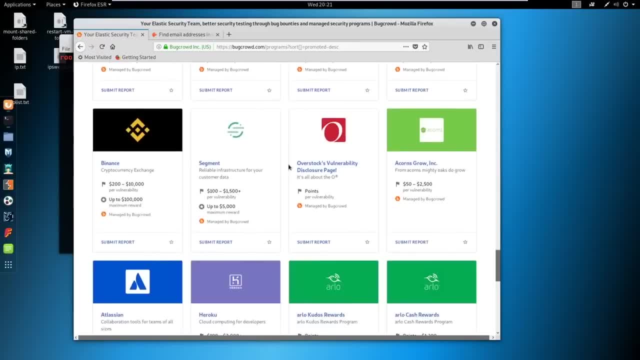 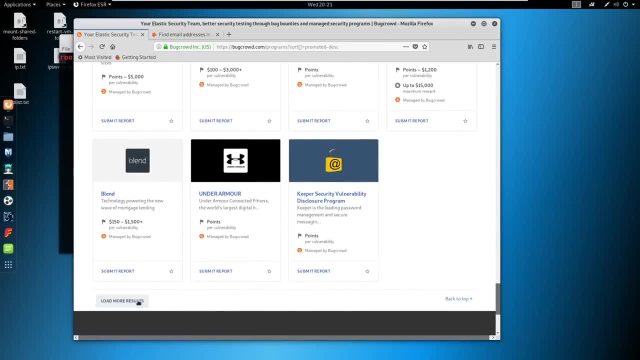 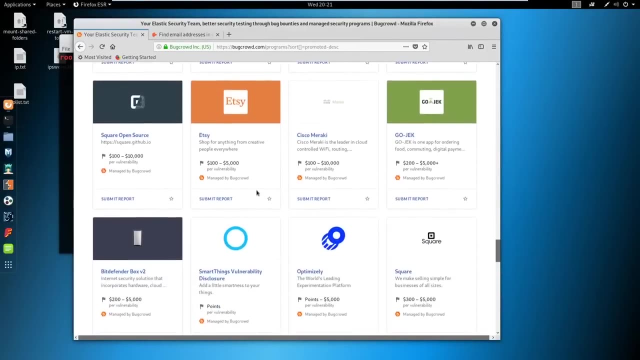 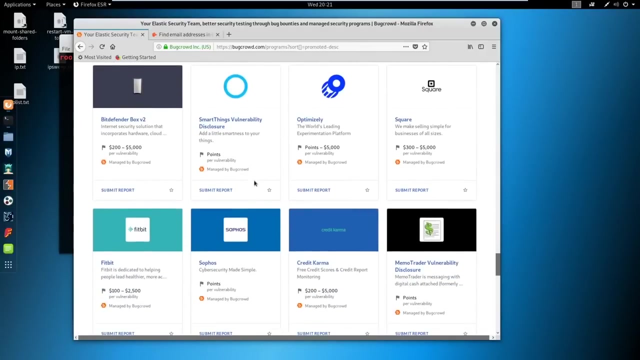 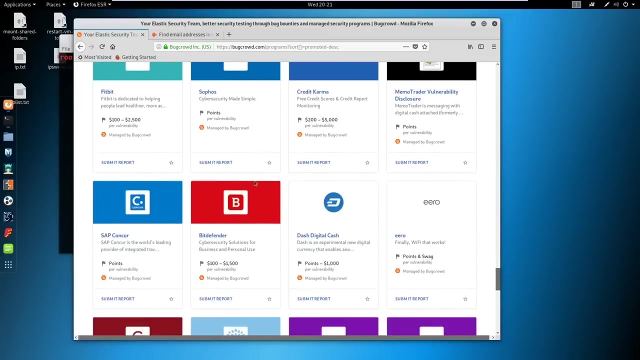 Um, but any of these would be be pretty good clients here. Tesla sounds good. Uh, we can do Tesla if you guys want Pinterest. We're not getting a. I need I need two votes for one thing, and then we'll we'll call it. How about that? 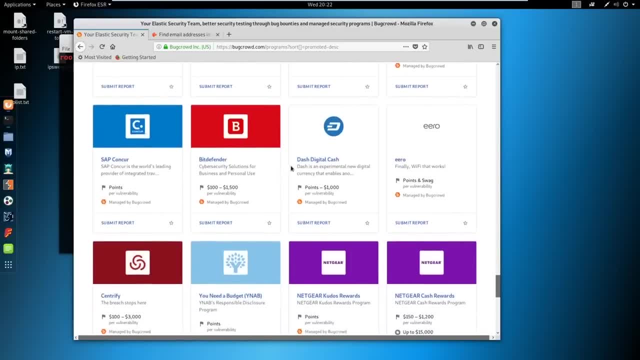 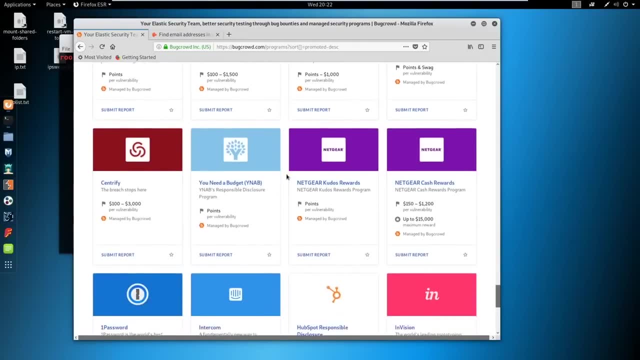 But we're taking the DOD out of this. Davey's being cheeky Tesla. You guys want to do Tesla? Okay, We'll do Tesla, All right, So you guys are going to do your own OSINT while I do. 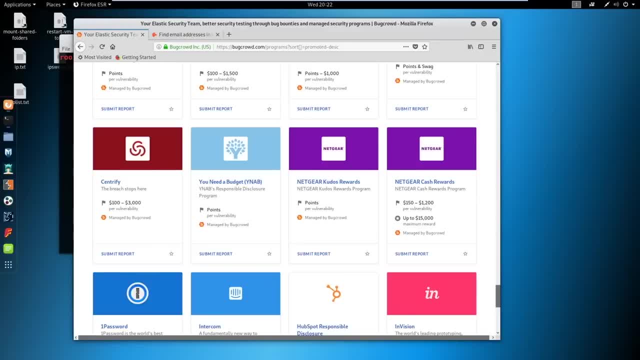 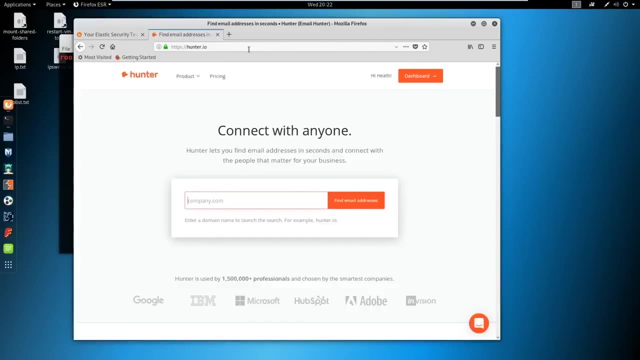 OSINT as well, but I'm going to show you. follow along, see if you come up with anything interesting that I don't come up with. Um, so a few things. one I've already got up here, If we look. so if you want to go create an account, go to hunterio. 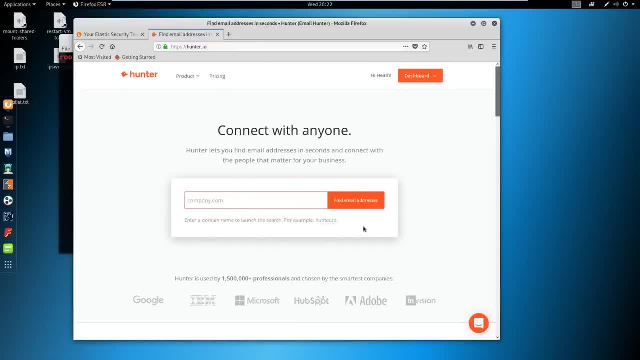 Basically, this will tell us: uh, we just enter a domain name and it'll search through email addresses and try to find people with that email address. Um, I think you get like 20 free searches a month or something like that. If we go into pricing, you get 20 free a month. 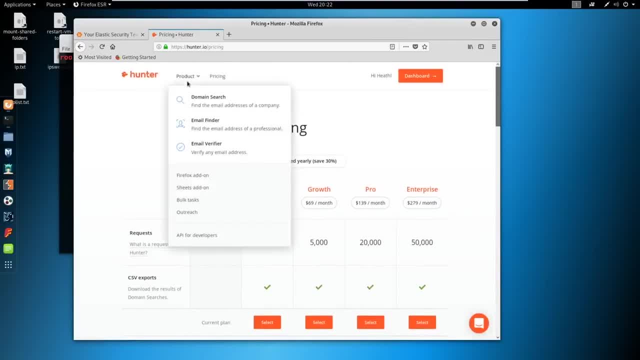 That's plenty for what we're doing tonight. Uh, you can also use an API key with the harvester on this and some other tools. I think Bluto has it now too, where you can use hunterio um and use one of these API keys. 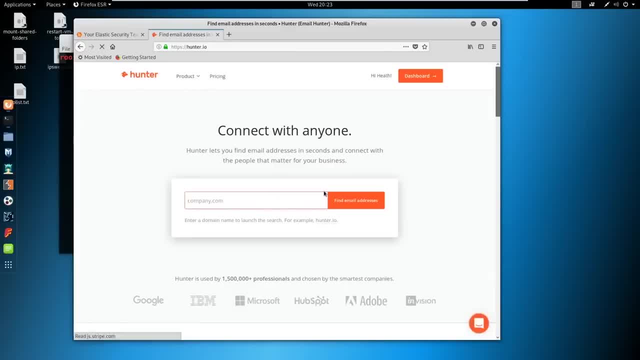 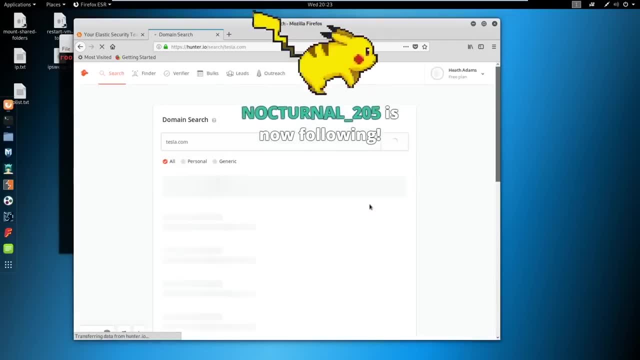 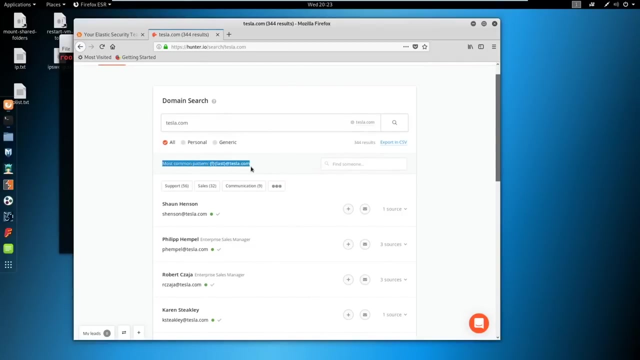 So we'll go back and what we're looking for is just information here. So let's search teslacom And what we're doing is we're looking at what type of pattern do they have, right? So we've got the most common pattern first, last at teslacom. 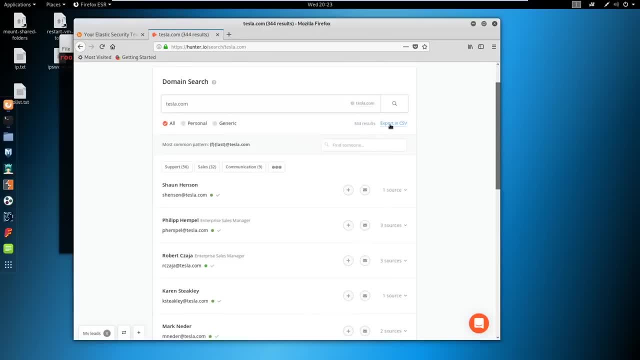 And if we scroll through, it looks like we've got 344 results. We can export this to a CSV, which is useful. Um and yeah, if we're searching through it here, we definitely see we get some job titles sometimes, right. 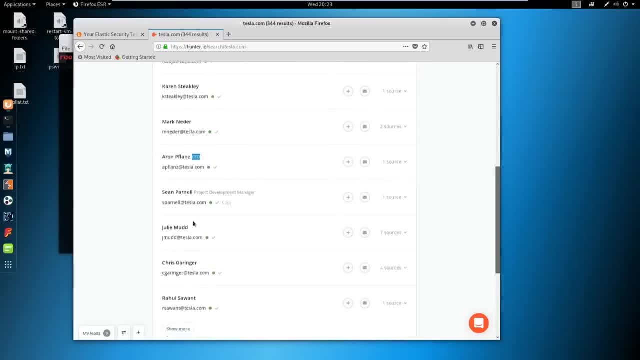 Um, we get- okay, it says CEO here, but we get email addresses of potentially interesting people, And what this allows us to do, too, is enumeration. Um, if we know for a situation here, it's not always true- but say we have a login interface and a lot of times, um, 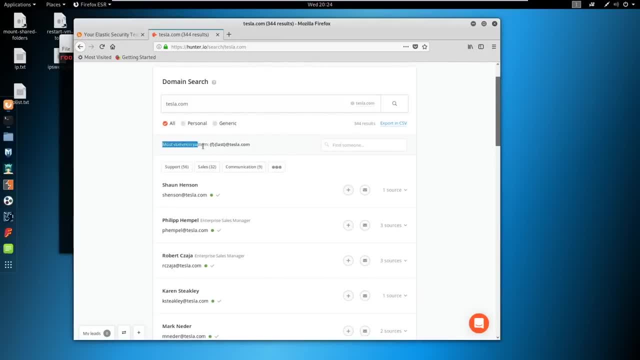 something like outlook, right, Say, we know just the common pattern, We don't have 344 names. but we go to outlook and we tried who? um, we tried to enumerate usernames through that, because outlook web access has a feature where it's a timing delay. 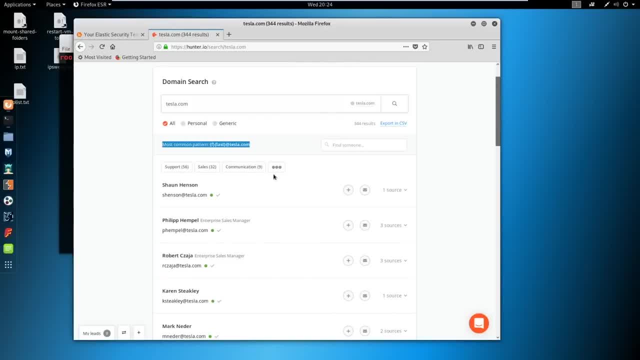 If the username is valid, it will come back pretty quick. If a username is not valid, then it won't come back right away. And there's that timing delay that allows us to be able to enumerate users. Um, we could take common first initials, common last names. 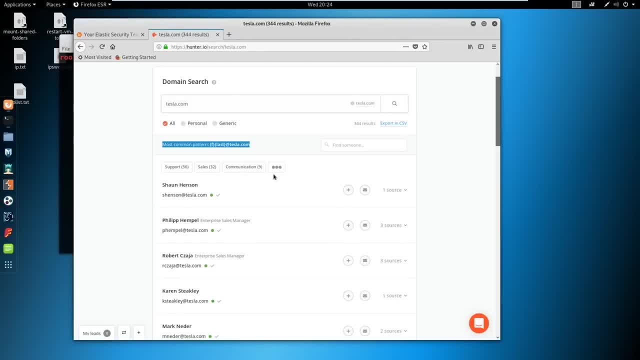 put those into a list and um, heave some of that at this search, If we wanted to. as an example, now, if they have limiting going on, which a lot of places don't, um, that will prevent us, you know. 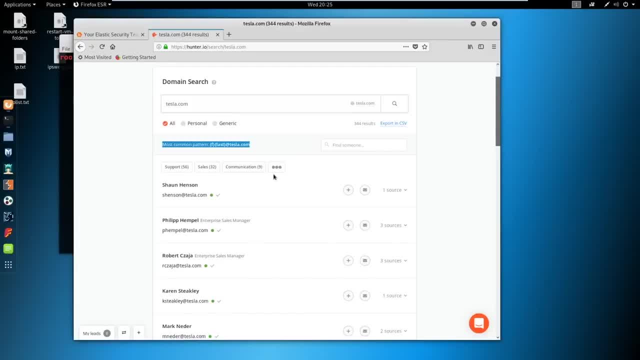 and if it depends how patient we are, if we're doing this on an assessment, probably not. If we're hacking and trying to be patient, maybe. um, these are just things to to look for, look through, Um, and with the time tonight. 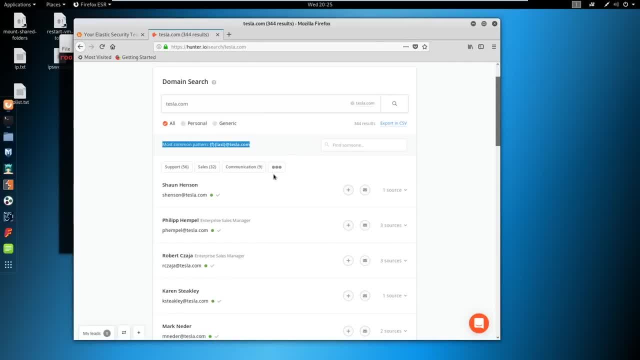 I see a lot of you guys are making suggestions in the chat. Um, definitely awesome, You guys can. can do that. I'm not going to touch on those as much, only because we've got a lot to go through in a little bit of time. Um. 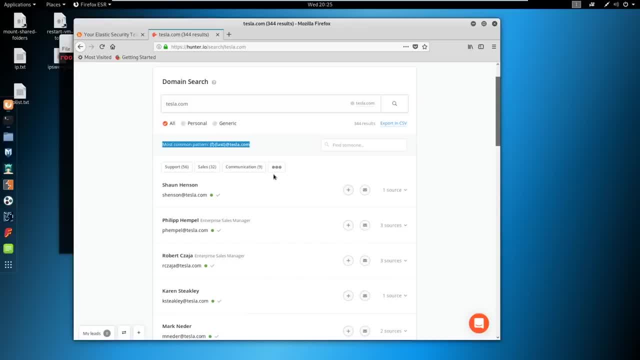 but definitely submit information, as you see it, and hopefully we can find some good stuff. Um. so for me, what I would start doing is gathering these names, Um, but somebody did mention that um looking through cred dumps, and I would 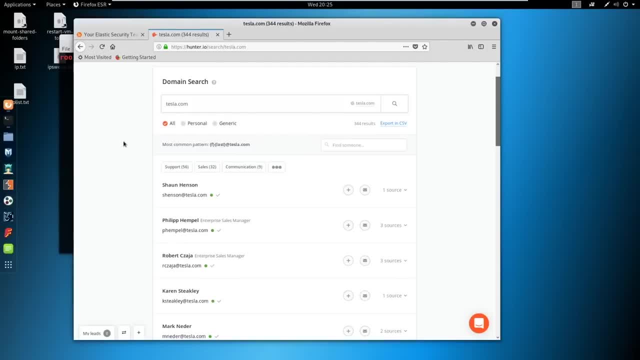 I was thinking about when I wanted to do that, when I wanted to show that off, but that is really the first thing that I do. Um. so basically, if you think about all the breaches and like the, have I been pwned collection right? Um? 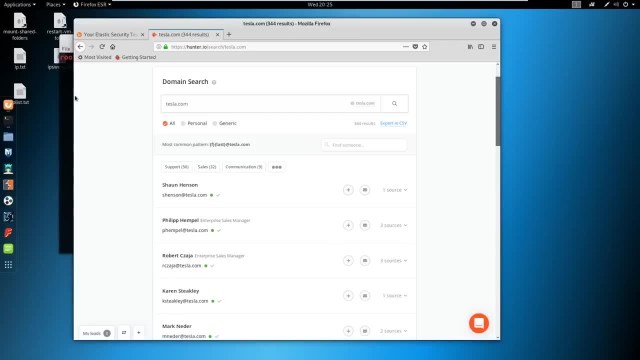 there is something out there and the list may be updated. And if you guys got an updated list, please send it my way because I would love to improve what I've got. But there's a 1.4 billion clear text password list- Uh. 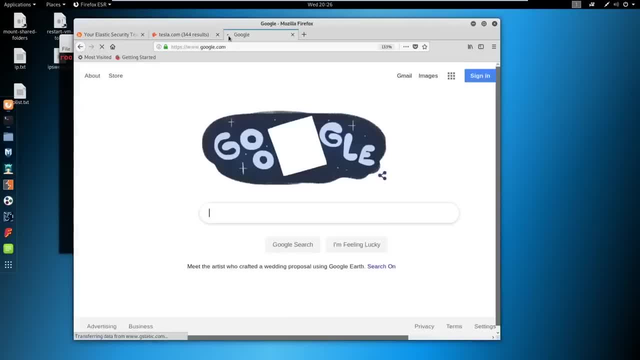 let's just see if we can Google it. If you guys are interested, I have the link. I just want to see if we can Google it. Uh, 1.4 billion clear text. I think it's a GitHub. Yeah, This tensor flow right here, this GitHub. 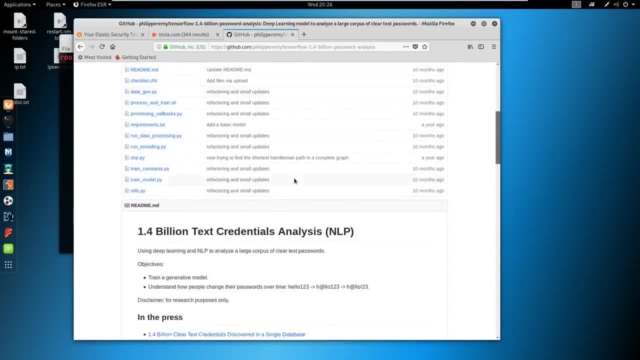 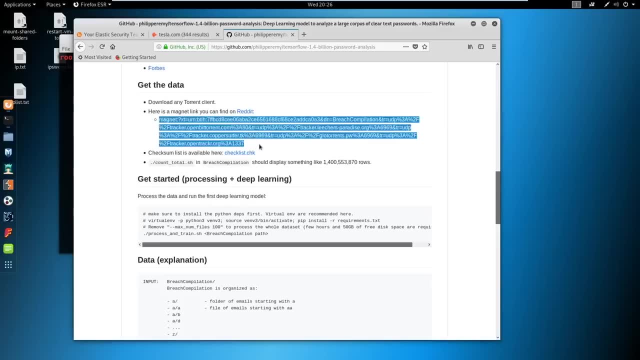 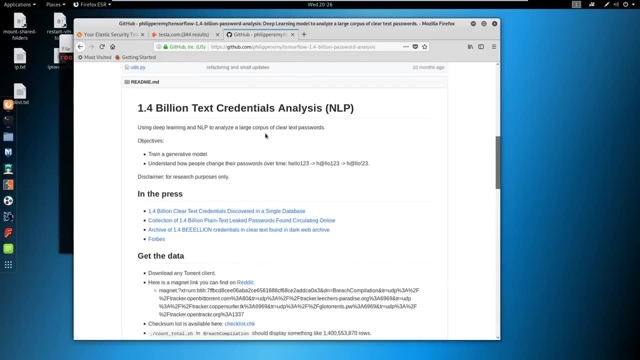 there is a magnet link in here. It's got plenty of people- probably the NSA- watching it, Um, but a lot of people sharing it. use copy this magnet, paste it, have your torrent and, uh, download it. It's 44 gigs, right, Uh? 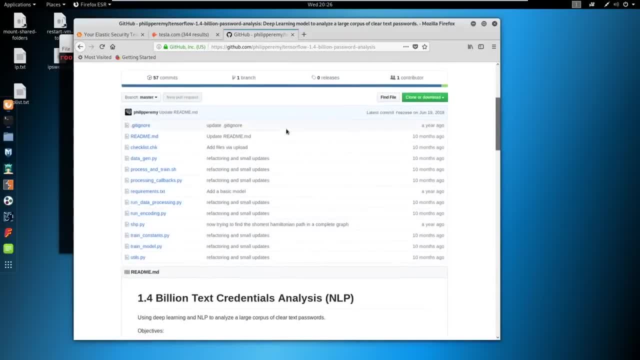 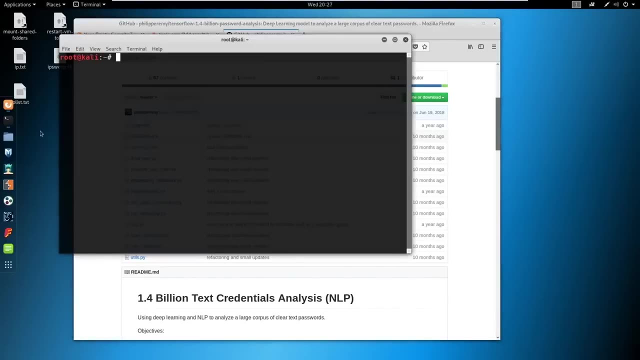 but what it does is it has 1.4 billion clear text passwords. So, um, not hashes clear text passwords. So if you build a tool to parse through these passwords, uh, you may be able to find some useful information. So let's look at something here. 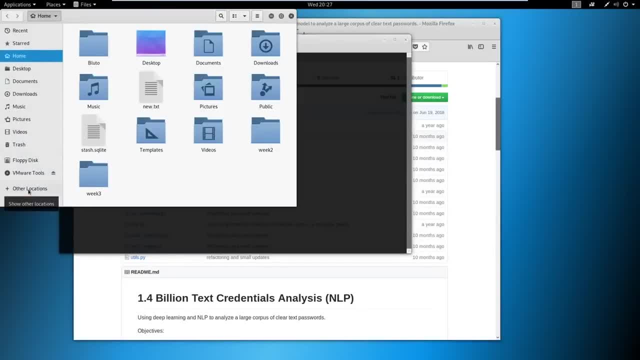 I'm going to go to my files and show you kind of what this looks like. If we go to other locations and I like to put things into my opt folder, So we go to opt and we go to. so I built this tool. 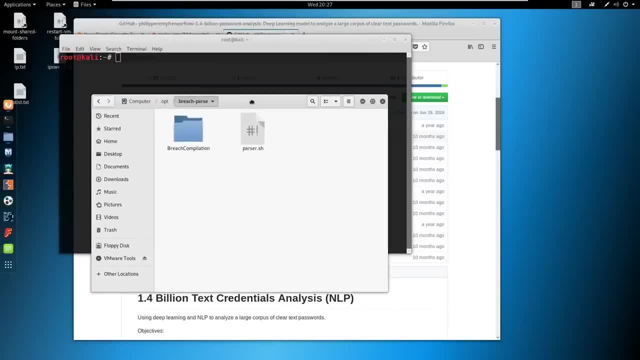 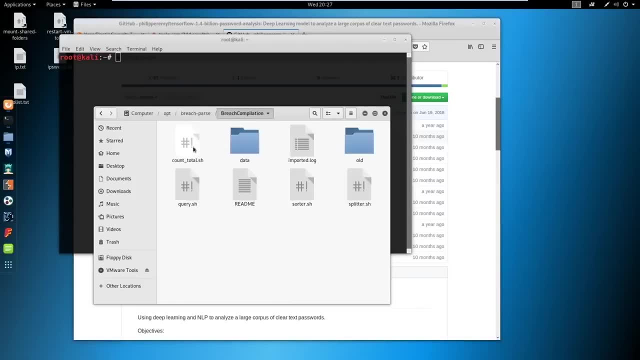 It's called breach parse, very basic bash script. It's all hard coded, nothing special. So you, when you download this, you get this breach compilation right, This folder here, and it gives you this data folder here and it has all these. 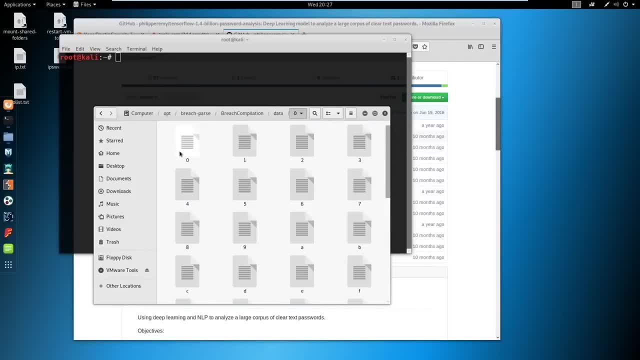 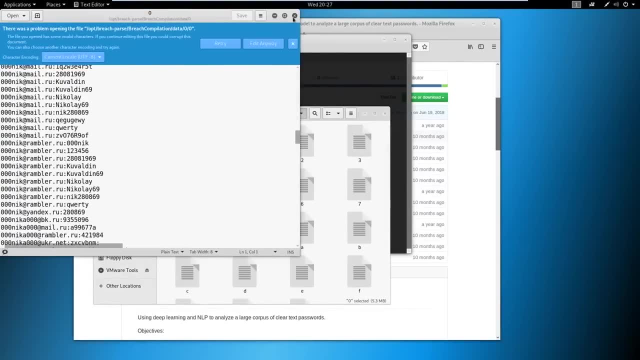 sub folders that you have. You click into here. you click on one of these documents, open it up and you've got usernames and passwords all throughout. Um, so what you, what you don't want to do, is use this for bad. 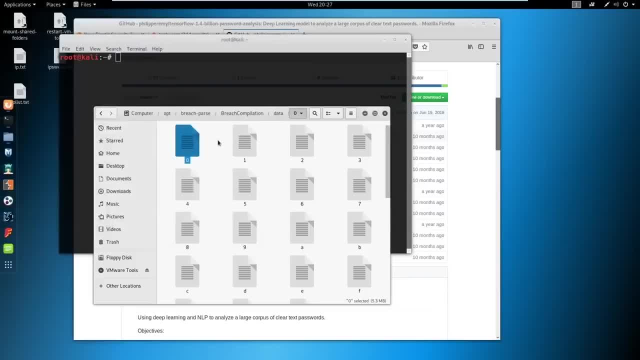 right This. there's definitely a lot of credentials in here. Um, I'm sure if you went to and pulled out something like all the yahoocom, you may be able to put that into burp suite, put that through intruder and get access to yahoocom. 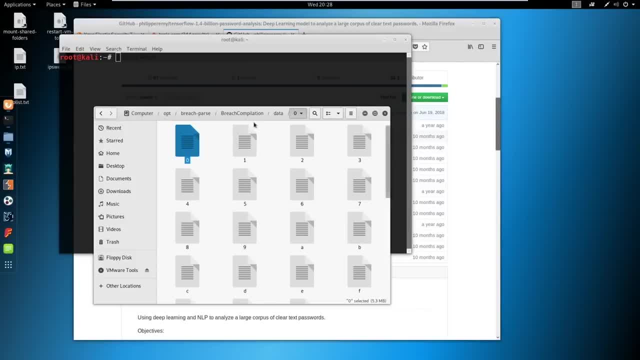 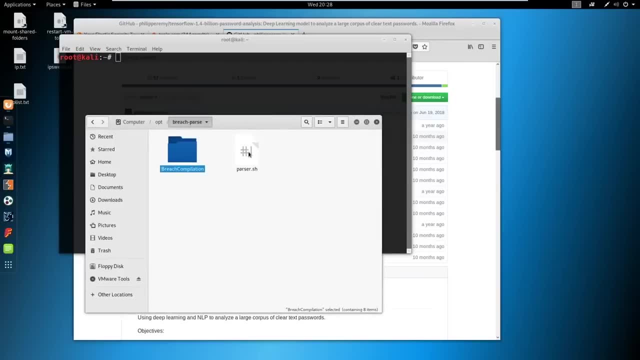 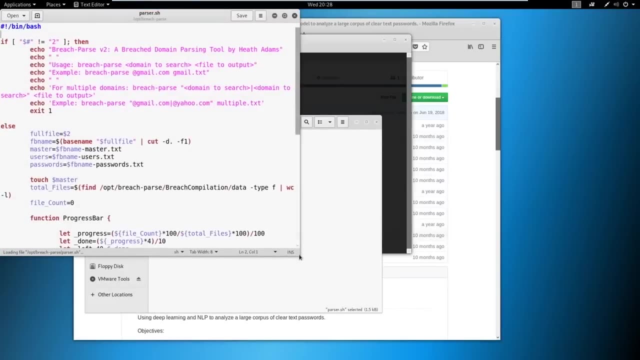 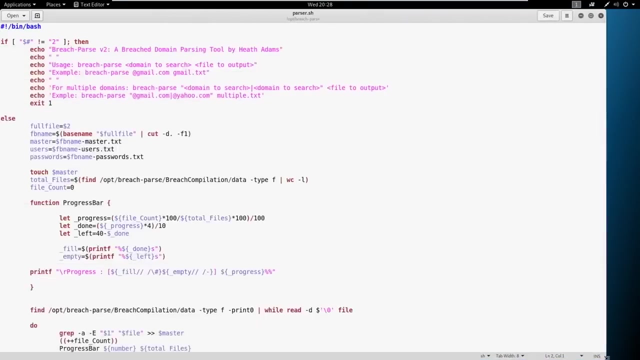 something like that: right, Don't do that bad. bad, We're going to use this for good. Um, so let's take a look at the script I wrote. Don't judge my script writing, please. Okay, This is a very basic script here and I just can we. 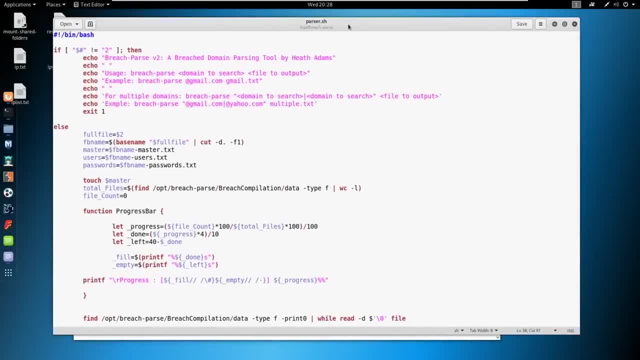 there we go, All right. So everything, uh, everything that we've been doing leading up to this has built up to this right. We did three weeks, basically, of scripting and programming and, uh, everything else in here. So this is a bin bash up the top, declared, you see, has an if statement. 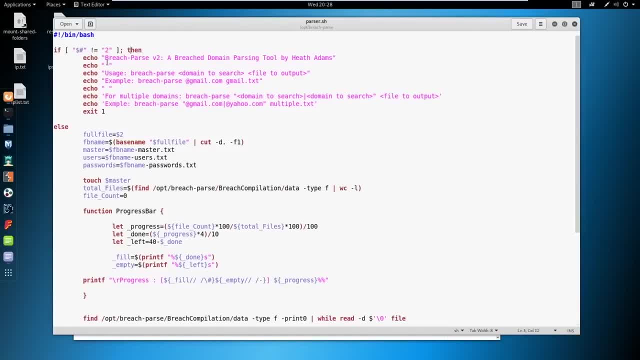 All I'm looking for is if there's two arguments. if there are not two arguments, then we're going to echo out the uh information how to use it and uh more usage down here. So basically the uses here is brief, part breach. 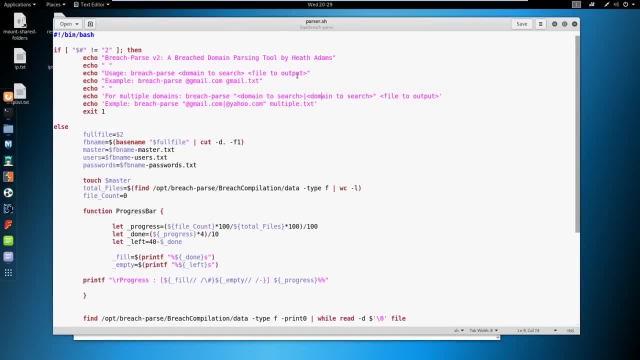 parse the domain we want to search and the file to output. If you want to create an in python, more than welcome. I will paste this script into the discord server And you guys are more than welcome to use it, Modify it, improve it. 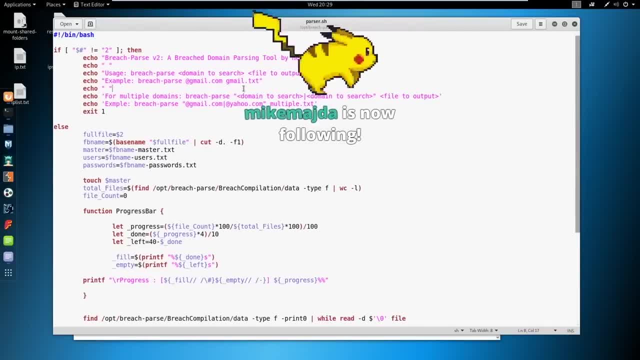 please. Uh, improvements are great, So, um. so basically we come into here and you see, if we want to do multiple domain, we can search like add Gmail pipe at Yahoo, and then just put it multiple dot text. Um, and then we do an else here. 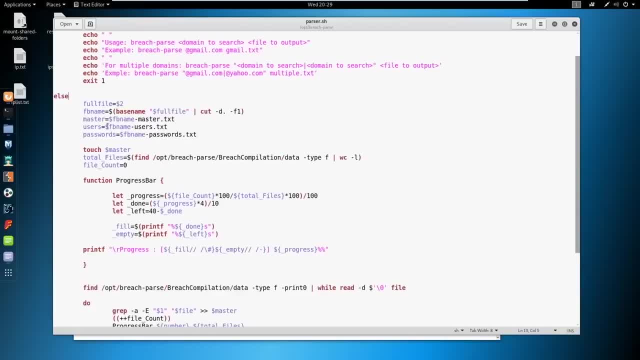 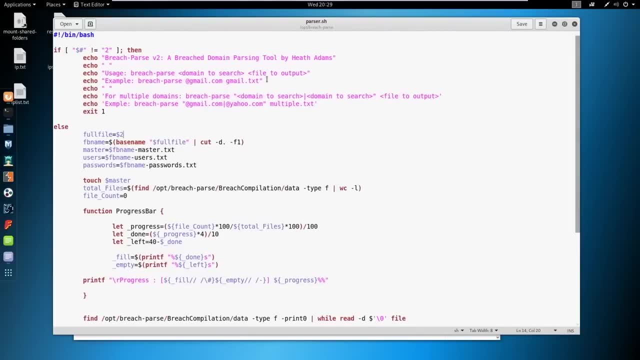 which you probably could have put into a function, but I'm a terrible programmer. Uh, basically, we are creating some variables. I create a variable full file here and set it to the second argument, which is this: Um, basically, what I'm trying to do is parse out if they put something other than dot. 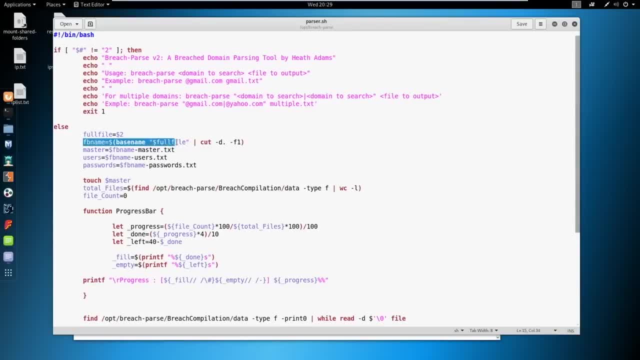 text. we're going to make it dot text ourself. Uh, so we take a base name of the file, we cut out the period and then I put it into three files. So there is a master file, there's a user's file and there's a password file. 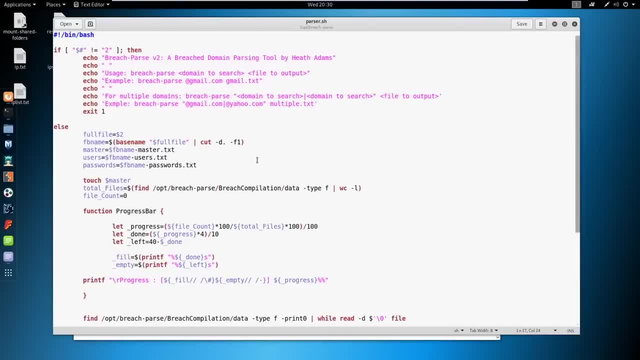 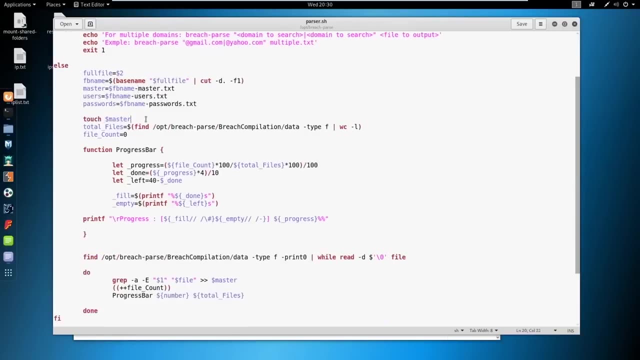 If you looked at when we were in that text document, it was a username colon password. So just to make it friendly, I've split it out into three files, but also kept the username colon password in a master. Um then what we do is we touch a master file here and we set a total file count. 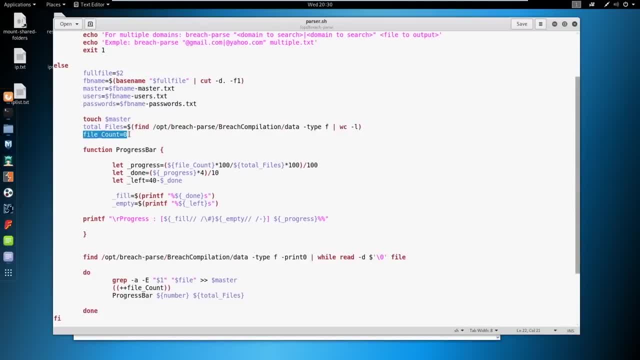 here by counting it, and we have a file count currently of zero. The only reason we do that is because I put in a progress bar. that way it can count how many files we have counted and then what total file number. we have to count a percentage out and know where the heck we are at. 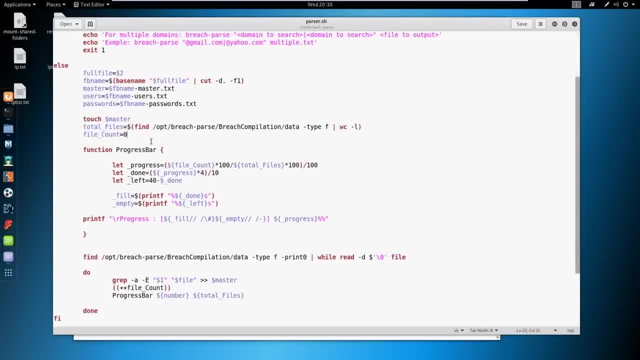 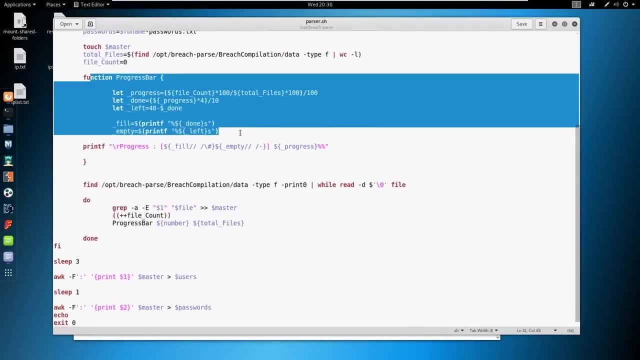 Uh, cause when I first built this, it was running for 10 minutes and I had no idea how close it was to finishing. Um, so this is a function bar that I stole somewhere and just updated for my own personal needs. And then what we do is we basically find: 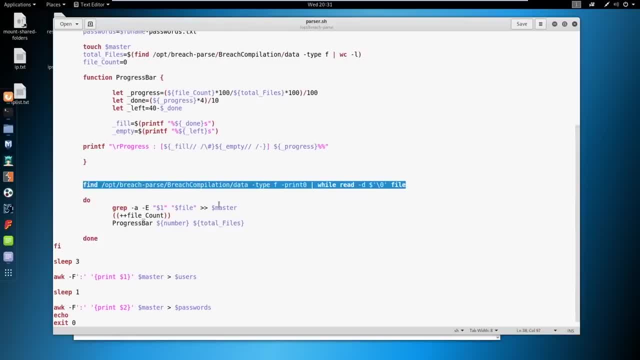 uh, every single file that's in every single folder, and we read through those, right? Uh? so what we do is a little loop here, We grep through those and we write whatever we find. that dollar sign one. This is our first argument. 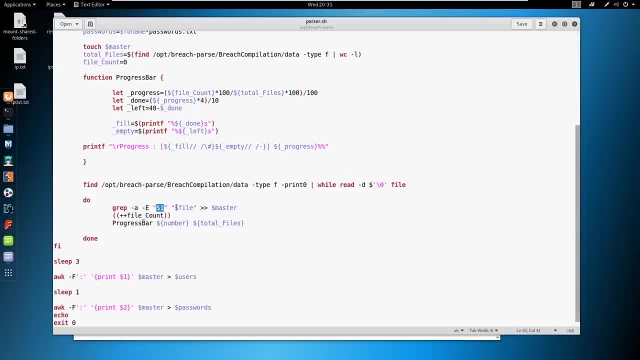 So if I say at teslacom, it's going to search at teslacom in the file and then it's going to print it out to this master file, Okay, Then it's going to increase the file count by one. This is for our progress bar, and then we're done. 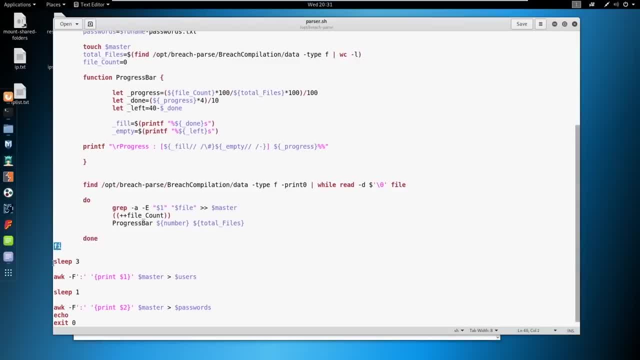 We end our if statement here and then we take a little nap for three seconds, Um, and then we do. all we're doing is this is print dollar sign one. We're grabbing the um, the users here, and then we're grabbing the passwords. 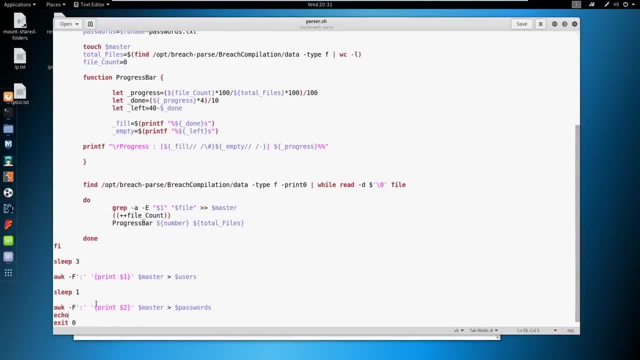 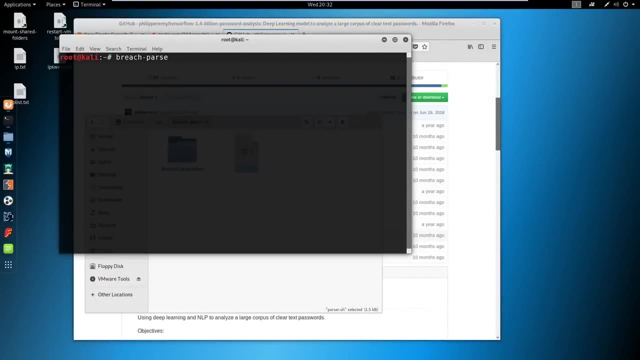 Uh, and then we exit out and we are done. So we're going to go ahead and let this run. Take a look at what this looks like, and I've created an alias for it. So it's just breach parse, and then we're going to say tesla dot actually at teslacom, and then we'll just save this to teslatxt. 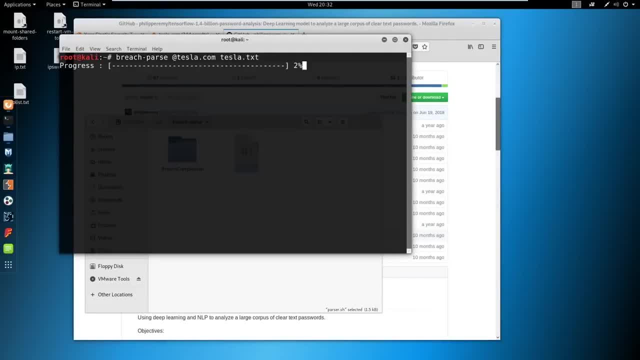 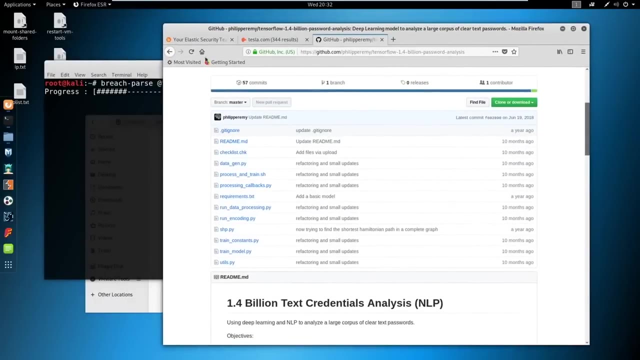 but it's going to strip the dot text off, Anyway, and make it its own thing. We'll let that run And what you'll see is we're not going to get back. Um, I've already done this search. I'll get back a ton of results. 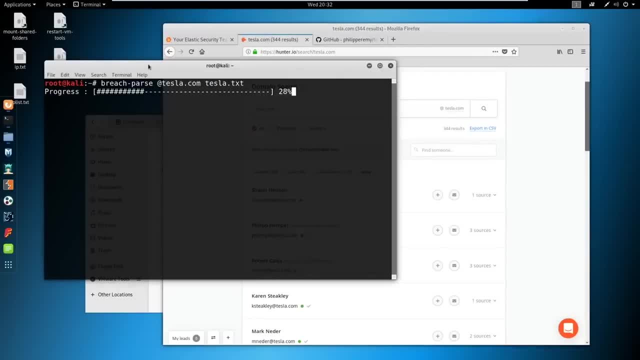 but we will get some results. Most of them are kind of they look iffy. Um, it's more promising. on on other assessments, Tesla is pretty Locked down. Uh, but when you look at a client, like the debrief I had today, 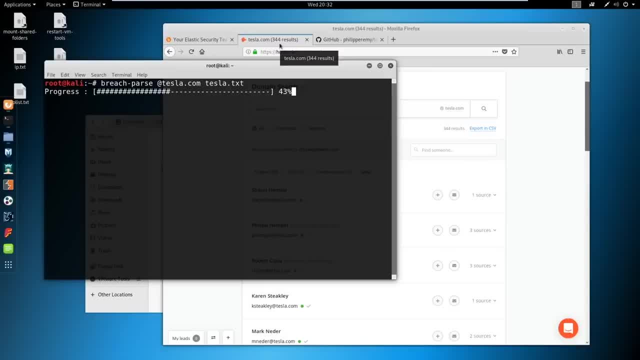 they had 900 and something users on this list. Um, this is one of the easiest ways to to get in when we're doing OSINT, right? So we talk about outlook and we talk about the issues that we have. Uh, so say, we take this list and all we do is we pass it into outlook and we send it with the username and the password that we found. 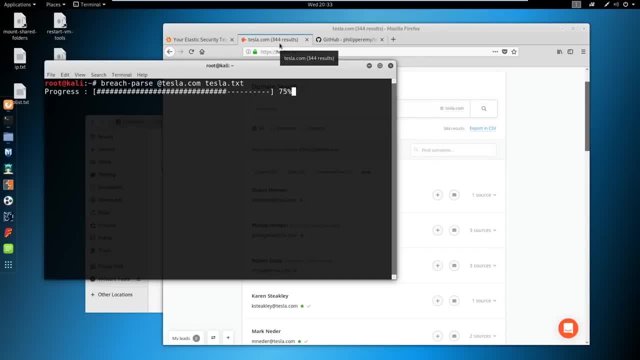 We could not at all have the correct usernames and passwords, right. Um, but what we can find, perhaps okay. say we do have the username password, easy, and we just got access to the email, At least if we don't have the correct username and password. 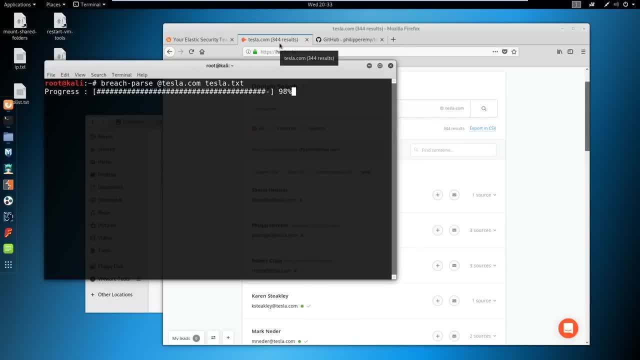 if outlook is doing some sort of username enumeration, then what do we have? Well, we know what usernames are good, What usernames are bad. We can remove the bad usernames, keep the good usernames and then we start throwing passwords at it. 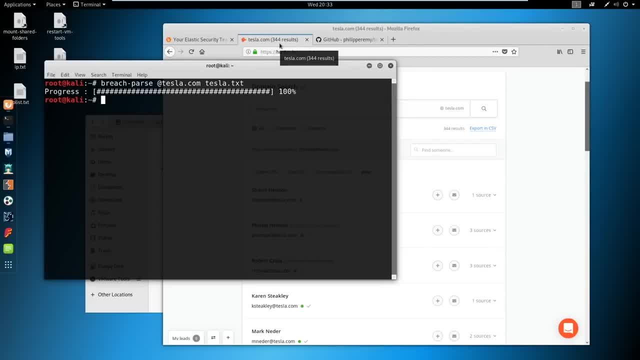 which is called Password spraying. Um, that's like winter 2018 exclamation point or spring 2019 exclamation point. uh, password one or the company name, like Tesla, one, two, three. So basically, you're looking for some sort of password that might get you in. 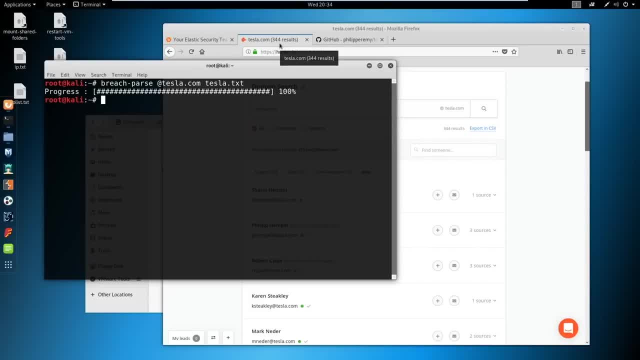 right, Um, so if they're not doing any rate limiting, that's an issue. Another thing that we can look at when we're in these documents: uh, I like to look through it and I like to see, because this isn't just grabbing a single user. 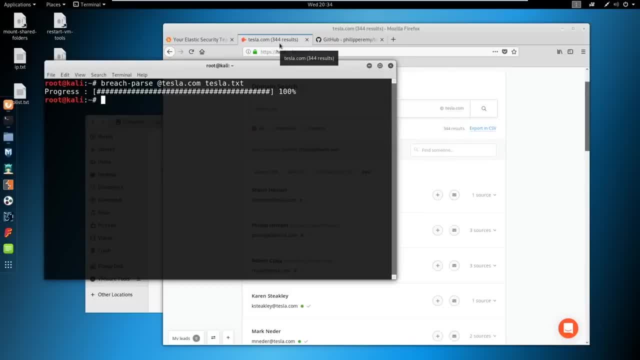 It may grab the user five times, that the user has been breached five times, And what we see sometimes in there is we see patterns. Their password may have been Jason one, two, three. Then it may be Jason two, three, four. 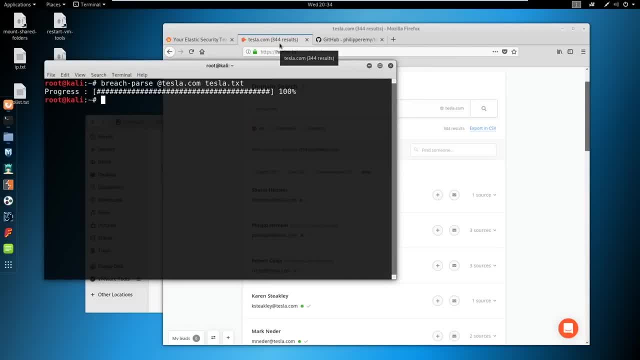 Jason. three, four, five. Okay, I know their pattern is probably their name or the name, Jason, with three numbers on the end of it And in some sort of incremental order. that has gotten me in before as well. So these are the things that you need to think about. 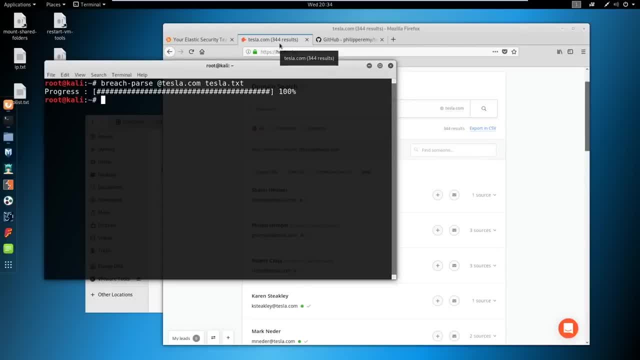 When we're doing OSINT in terms of password gathering off breached list. we're going to talk about this way more heavily. I'm just giving you the concepts and what things to think about, Um, but these are the things that we'll cover later on in the course. 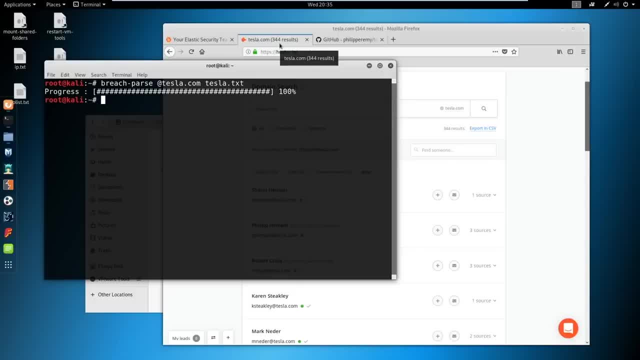 When we get into that situation where, um, we've tried everything else, there's no visual exploits, Everything looks patched, but we can still get our way in Um, especially if social engineering is off, um out of scope. A lot of times you'll have an external 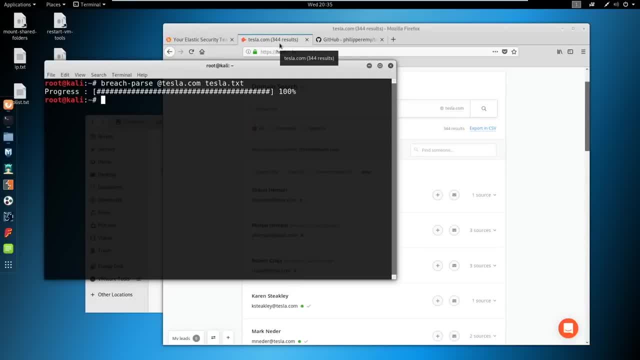 but social engineering will be out of scope. So if it's out of scope, then you're limited to what you can do and what you see, Um, and sometimes you don't get a lot on an external scan. So let's go ahead and just take a look at what we've found. 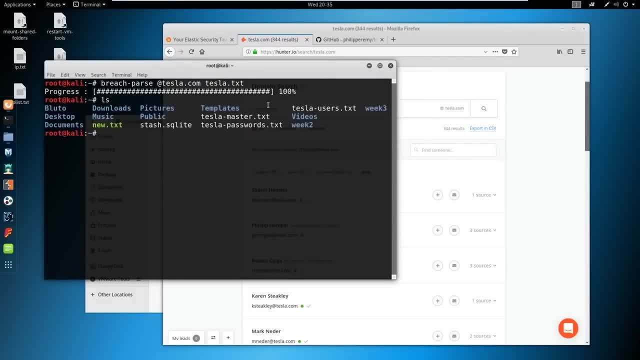 So if we LS here, you'll see that we've got- uh, we've got- the Tesla users, Tesla master and Tesla passwords. Let's just go ahead and look at the master. We'll just cat that out. So that's what it's looking like. 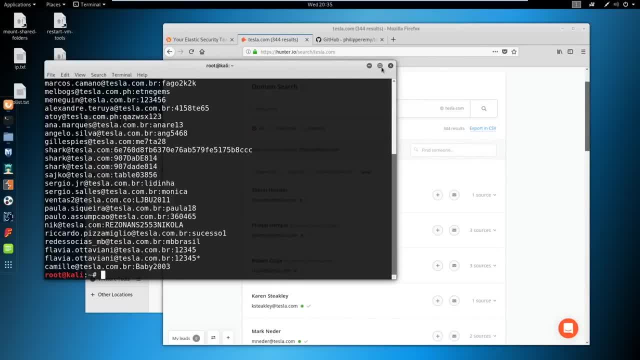 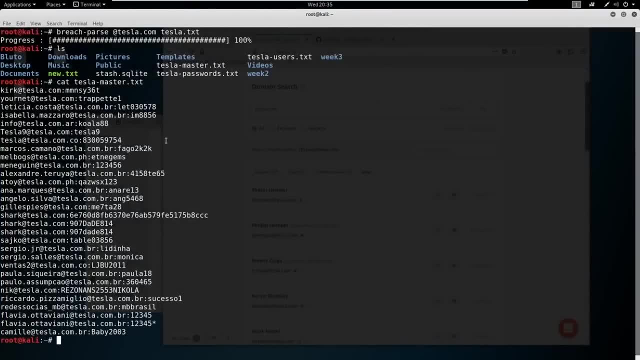 It's looking skilfully. red team is wanted. That's what's happening for your current engagement. They want red team, but not allowed to social engineer. Yeah, Then it's not really red team. Is it red team And pen testing, or two different beasts? 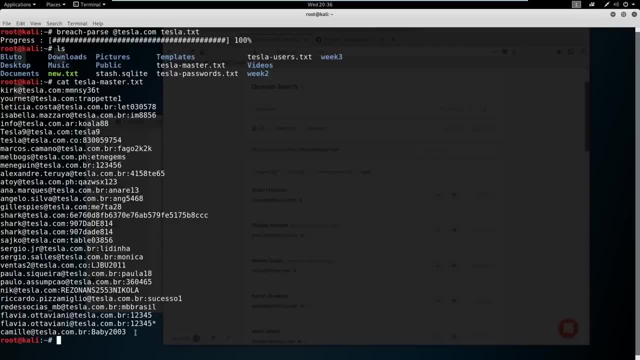 Okay, So we don't have a lot here. We we really don't, um, and what did we see before we saw? we saw a user where first initial last name right, and when i'm looking through these, i'm not seeing any first initial last name. 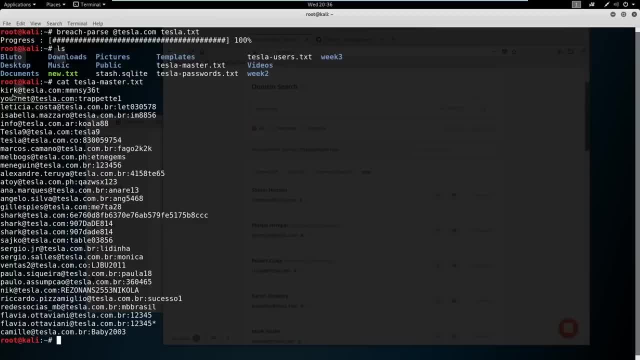 uh, you, you have first names a bunch of times: kirk, leticia, isabella, this, tesla, nine. uh, the shark here. so this could be maybe an s? hark. uh, it looks like. maybe at some point. if these are true, it looks like at some point they had a first name option or they had a first name dot last name. 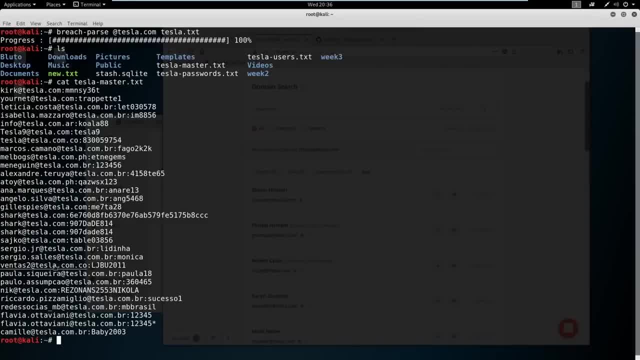 option, but i'm not seeing a lot of first, initial, last names. so we're getting some sort of mixed results when we look at the hunterio and we compare it to this right. so who knows? but our next step here would be to take these credentials and try to push them to through a login, if we could. um, and you want to look for? 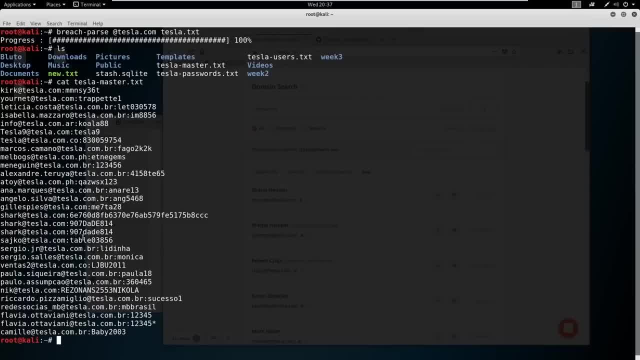 patterns right, like you see the shark at tesla. look at the 907, dade, 814. you see capitalize some things in there. um, it would not be very difficult to set a rule, set and alternate some of these letters with 814, 907 and then alternating dade somehow with uh capitalization. 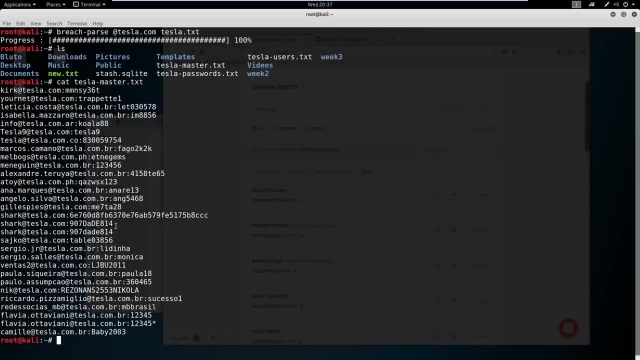 they're probably honeypot creds placed by tesla. that would be some next level stuff could be matured. email addresses started with first. last had to grow also possible. decoy creds are possible. so these are- these are the things we look for, though this is. this is my first go-to. 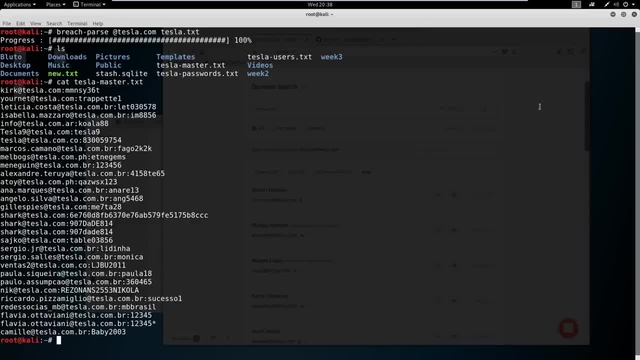 when it comes to oscent. so you guys were mentioning it, i figured i'll show you first and foremost. i'm going to show you the first go-to when it comes to oscent first. i was going to show you more towards the end, but okay. so we've gathered some information on what usernames might look like. 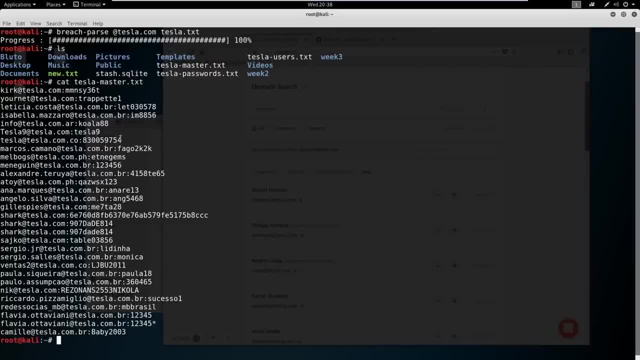 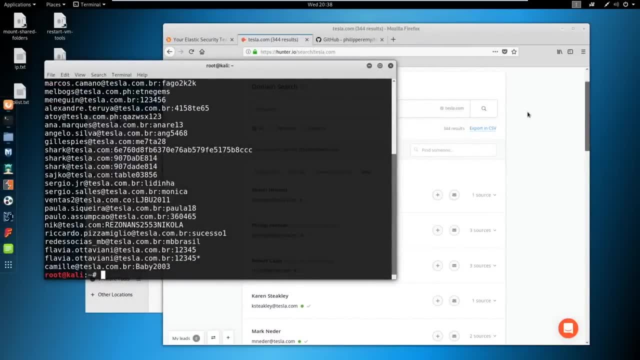 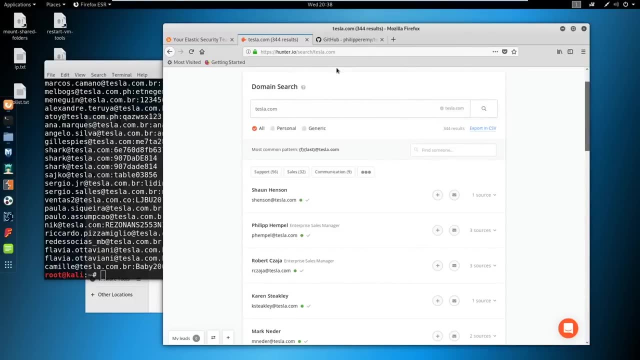 um, if we were to start attacking, we would use these credentials against them on login forms. but we're not attacking, we are just getting uh information right. we're doing reconnaissance. so what else can we do? well, i like to just go out to the website. that's one of my fun things to do. 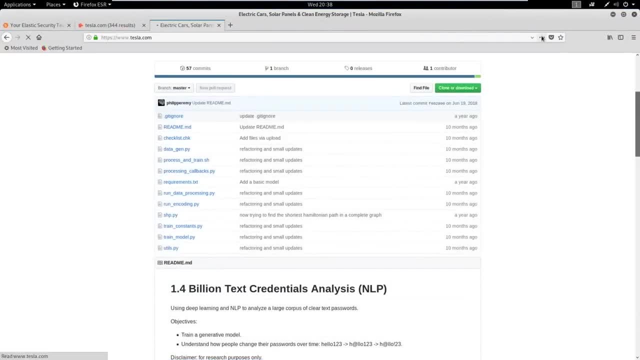 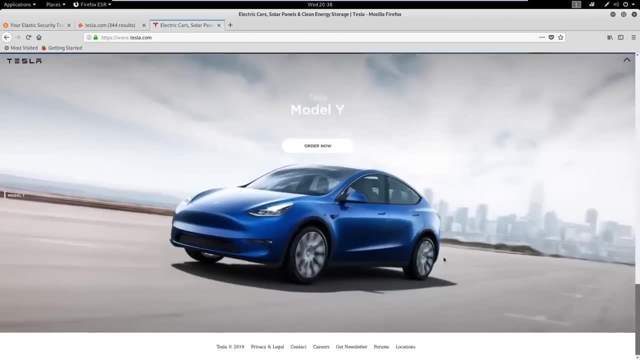 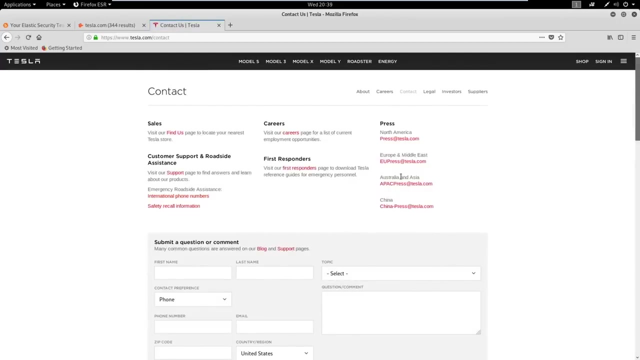 let's just go to teslacom maybe buy a tesla while we're here, or a roof solar panels. man, all right, i like to look at contact information, location information. so let's look at contact. okay, so you get some more email addresses here. press, eu press, whatever. 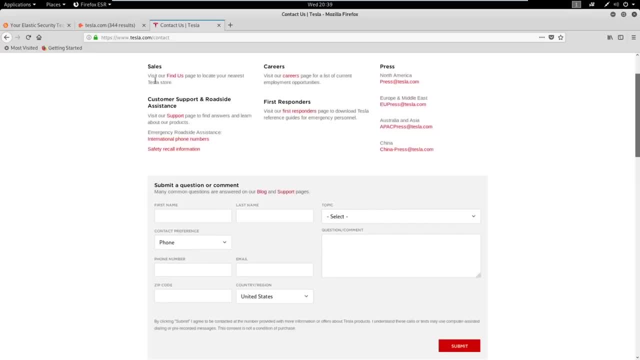 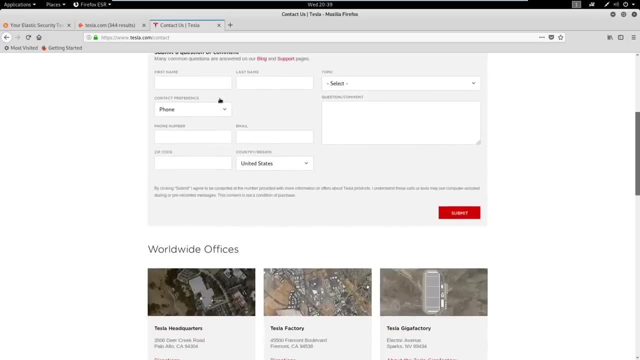 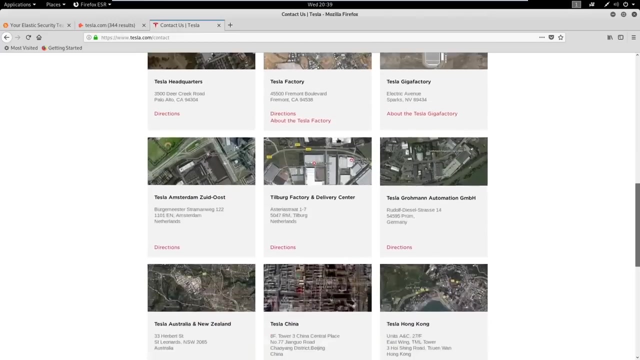 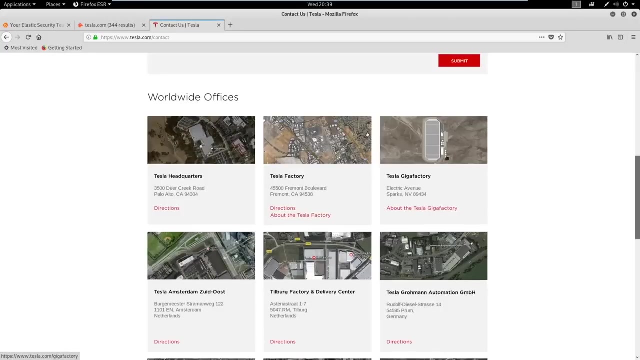 um, they've got store locations when you're trying to find your nearest tesla store. my next giveaway is a tesla 3. i'll need a lot more donations for that. okay, look at this though. this is cool: we have all of their offices. and not only do we have all their offices. 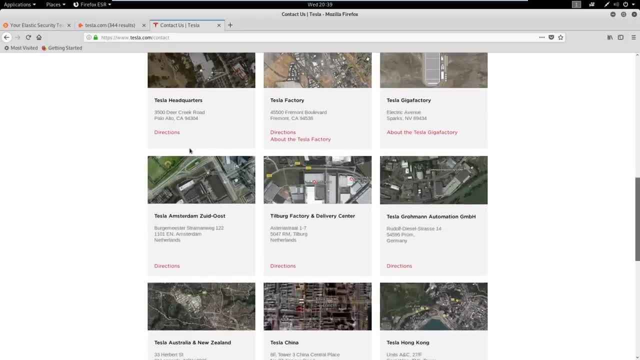 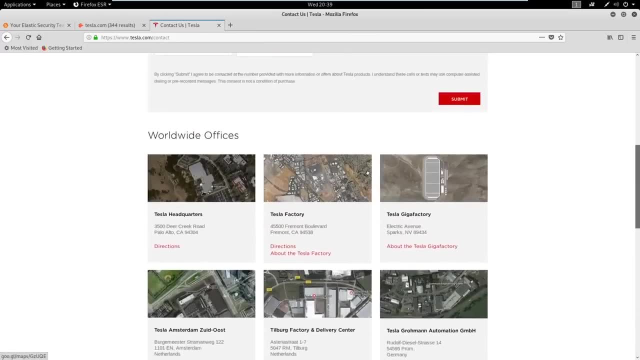 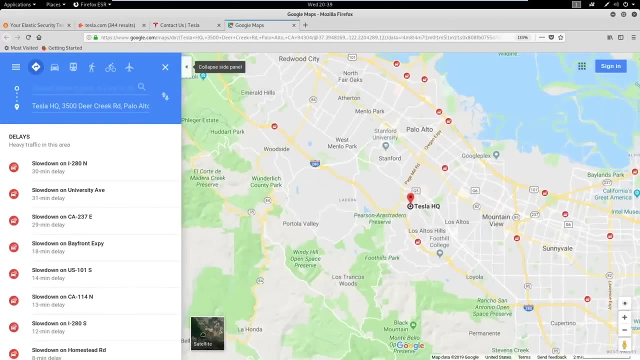 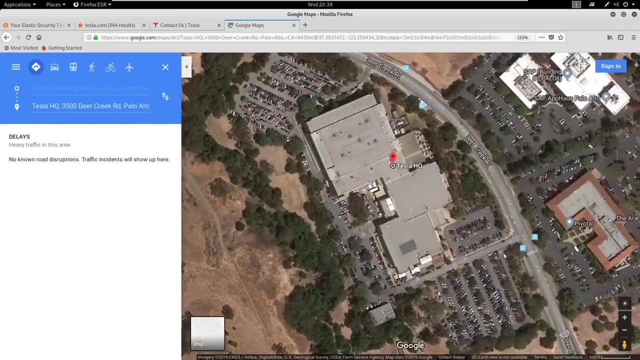 they have given us map views already, aerial views of them. that's pretty cool. so let's just click on tesla headquarters- and now i haven't gone this far in into the satellite or anything, so we're we're diving in a new, new territory here, so we want to zoom in as much as we can and try to find information that we can. 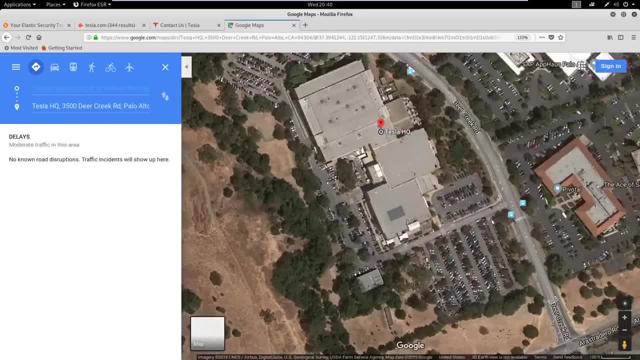 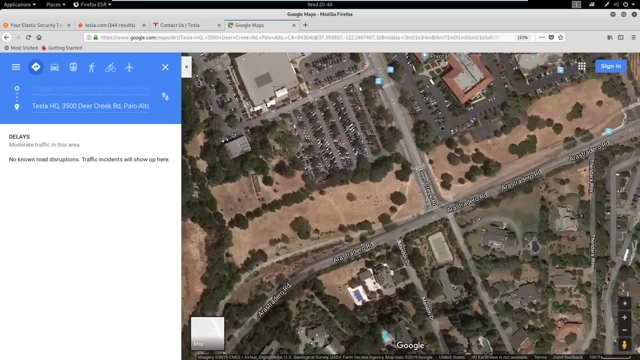 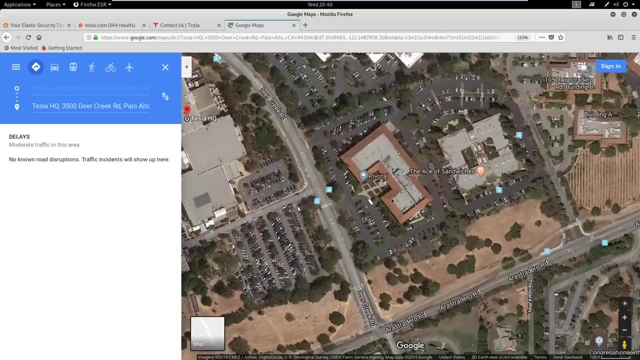 you want to know what their parking lot looks like. not only do you want to know what their parking lot looks like, you want to know if there is, say, like an adjacent parking lot or like a sandwich shop or something nearby that you can park. and that's what we do when we um say like we fly the drone around, right. 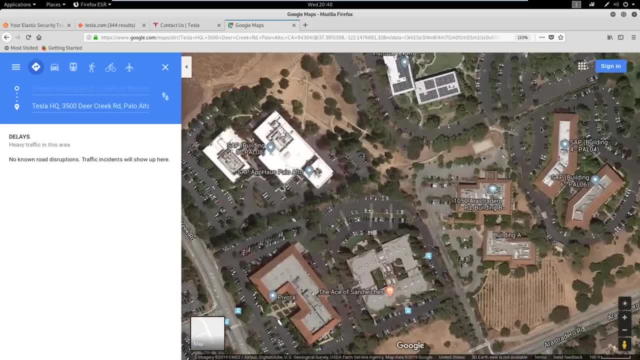 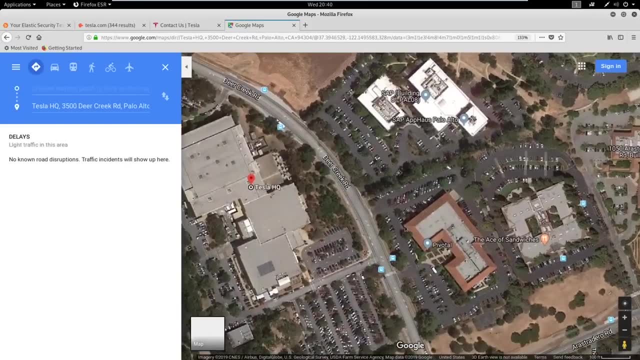 when my co-worker flies his drone around. we'll go park way over here. that thing has like a three or four mile range and what we'll do is we'll fly it over here. we'll take a peek at what's going on and see what we can do. 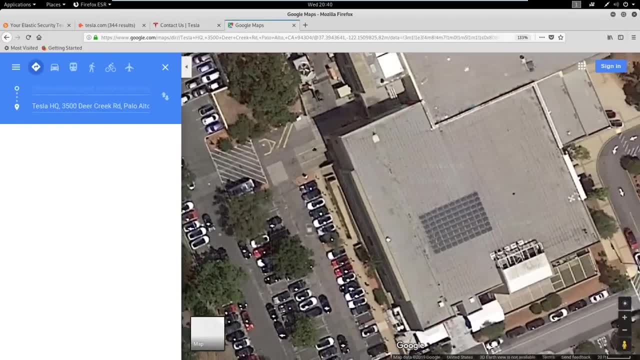 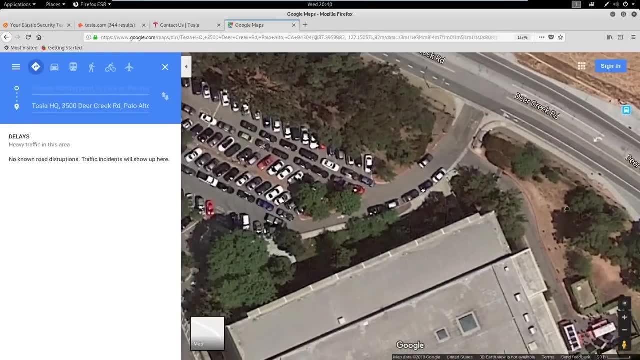 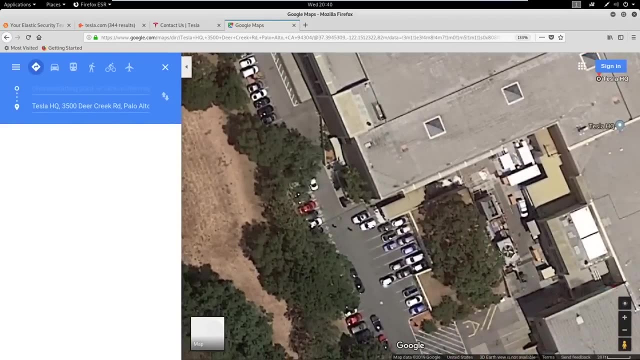 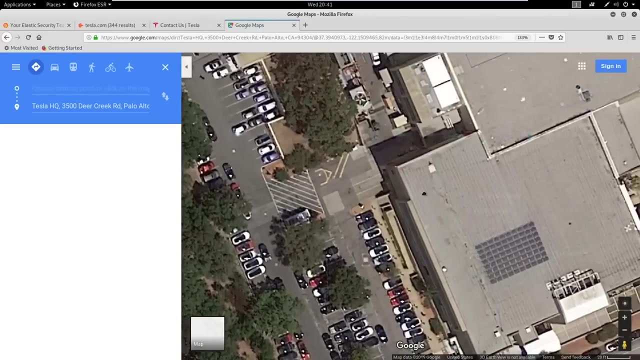 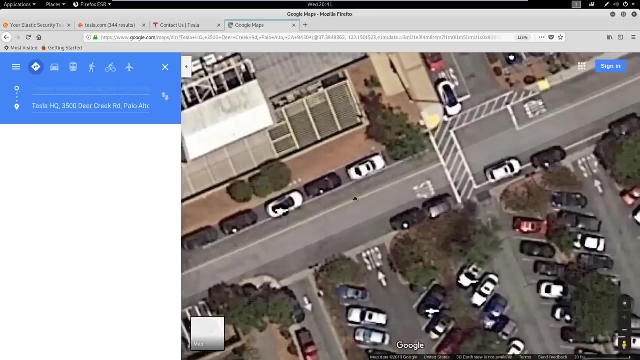 so we're looking for, for doors, areas of interest, parking. is there a security guard gate area that's on site? not really seeing that? so, yep, so we can just dig in as as deep as we can go. um, but eventually we'll get to a street view, and maybe sometimes street view helps too. 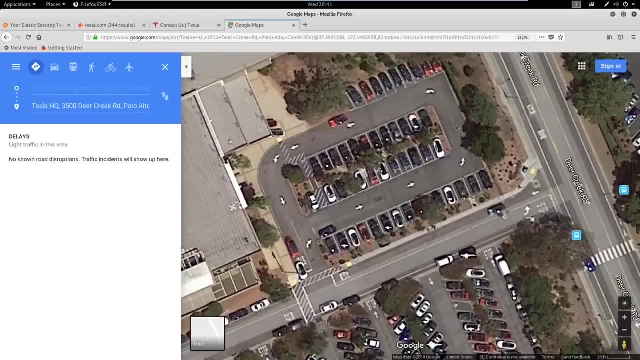 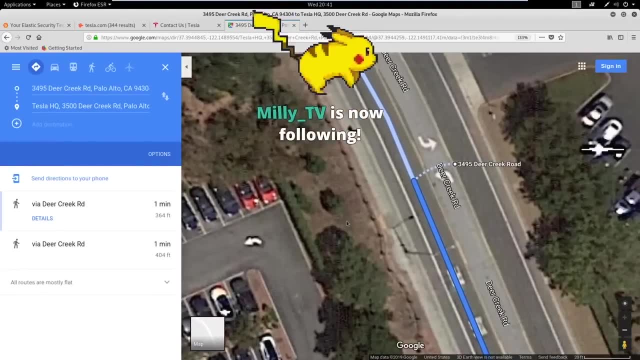 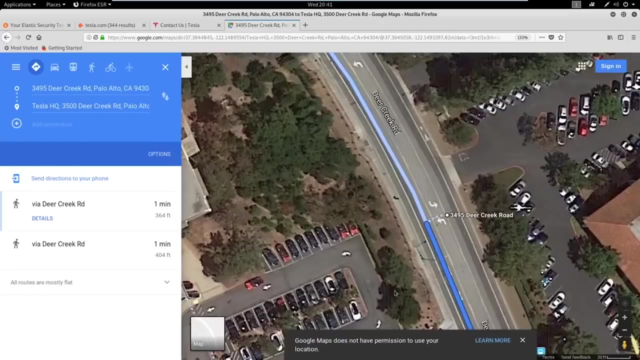 um, but we just want to gather as much information that we can about about them. let's see if we can double click on the street and get in here. i'm not getting a street view or i'm dumb. i don't want location access. so many teslas. 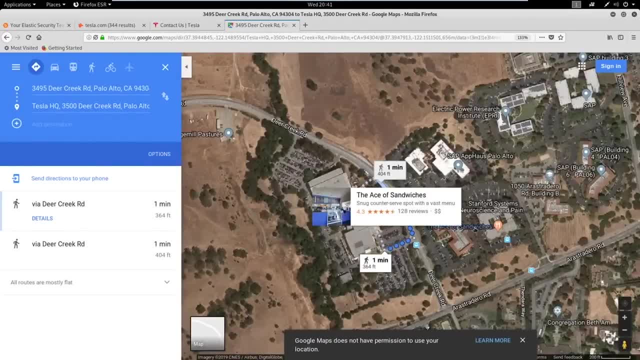 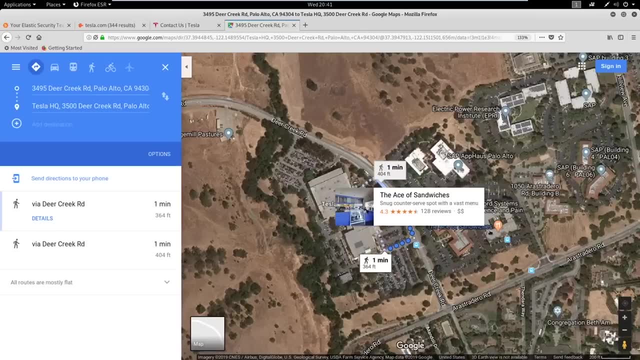 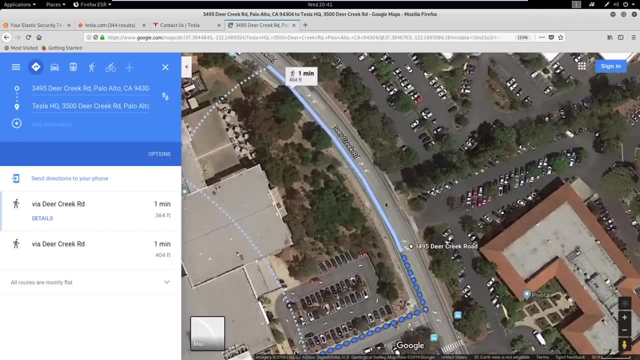 in the parking lot. yeah, that's strange, huh, let's take a look. oh, there is an ace of sandwiches. somebody said there's a sandwich shop across the street. literally this is probably where we'd park at the sandwich shop. so somebody said that, uh, strava is a. 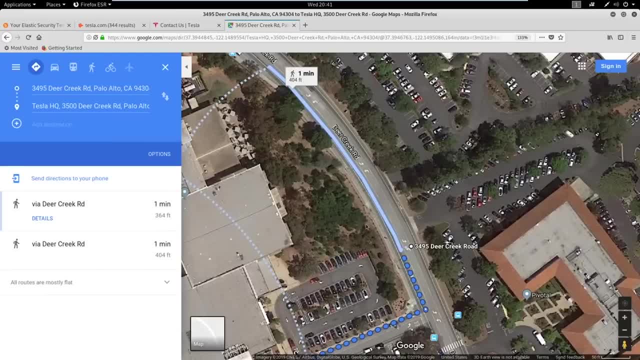 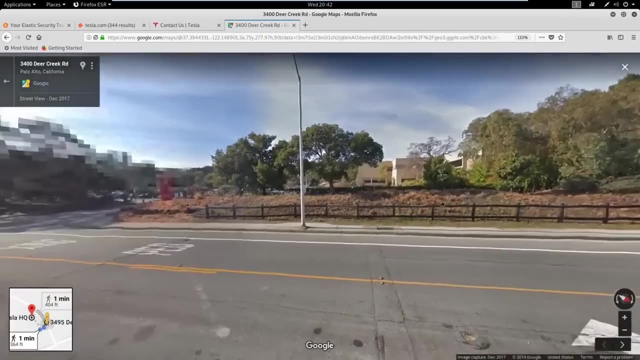 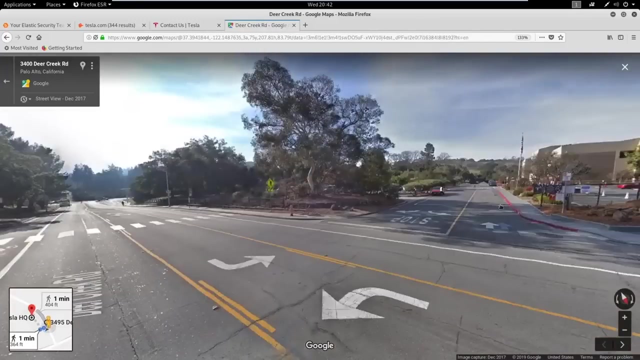 a pile of data. well, if you've got, you've got information, you should submit it for us, man. so drag and drop the little dude. this guy is all you do. i'm so bad at this. you guys are expert level, next expert. all right, can we get into this area here? doesn't look like it. no, 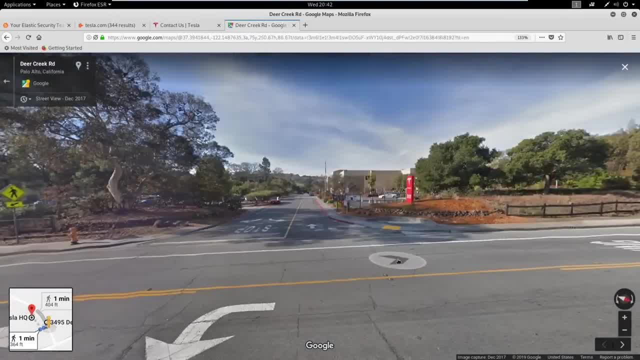 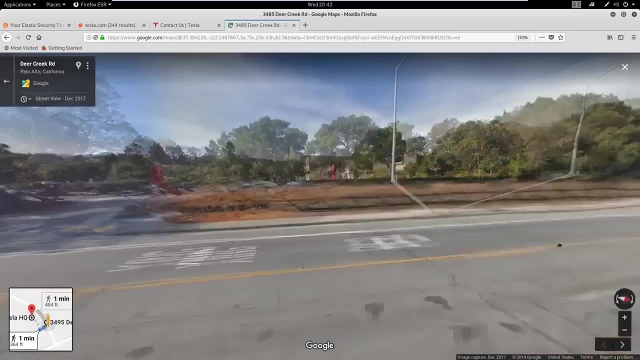 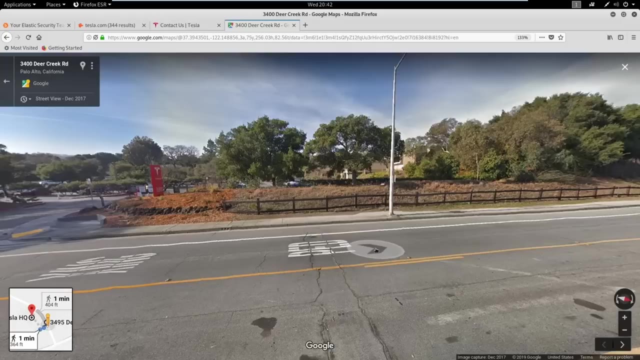 so what can we see from the street? doesn't look like a bunch here. it's definitely tesla, right and uh. sometimes, when we're doing this, sometimes buildings are new and you won't even show up on on google maps. you'll have to look at other locations. some sites are pay-to-play. when it 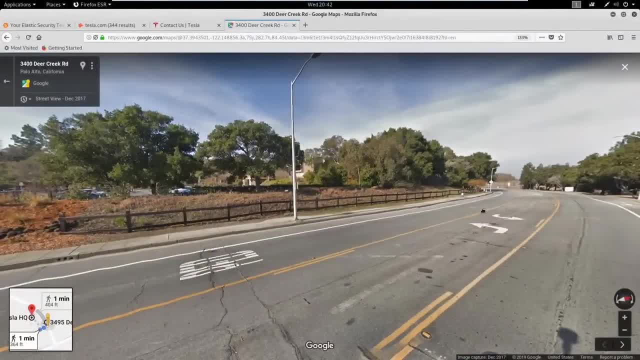 comes to satellite information, we did a a building physical of a building that just got built and wasn't anywhere, but we were able to find the information through a different satellite. but some of them are pay-to-play. but just know that google earth is not the only satellite. 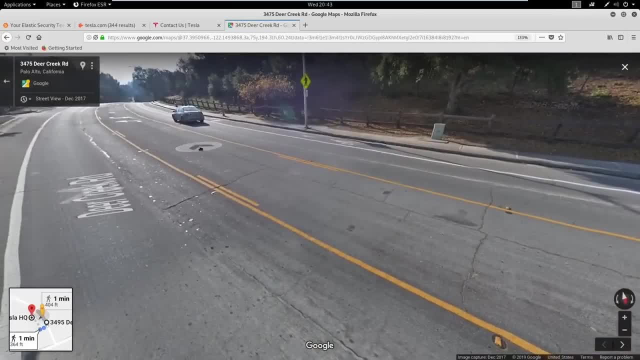 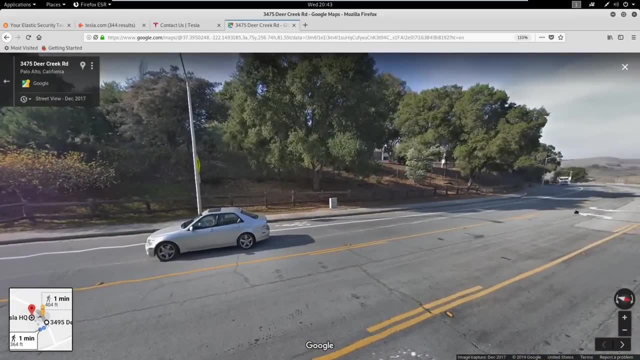 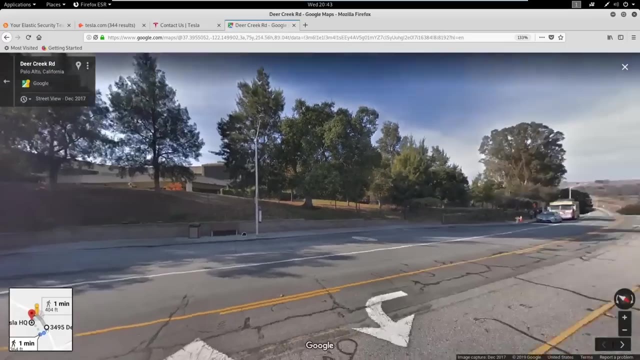 okay, what are the chances? this is a tesla. it's not a tesla, darn. uh, we can form around the back side, see if there's anything over here down the street. yeah, you really can't see a ton. there's not a ton of information here. 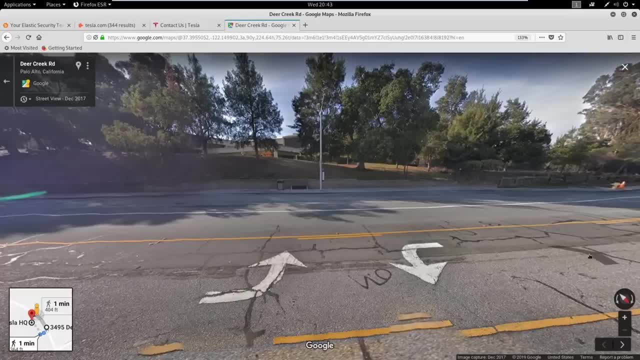 that's a budget car, what are the chances you could see parking tags? i don't know. it's a good question. so we don't see any sort of like big security which is a good sign if you're doing a physical right. they probably have badging in and out. um, i'm sure they have like a big security presence when it comes to. 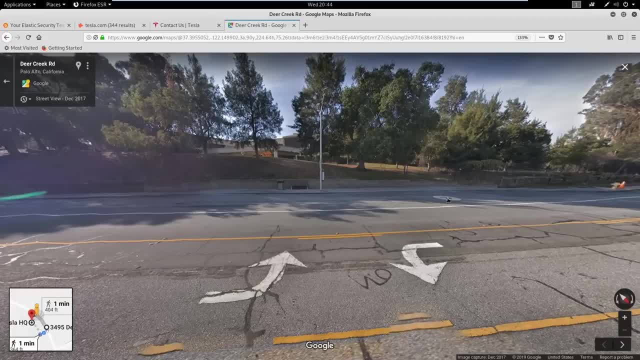 the front door area. they may have some sort of two-factor or anything where you need to get into anything of interest, right, um, but in terms of having to drive through and talk to a security guard to get past the gate, i didn't see anything like that. i don't see any kind of crazy fencing. 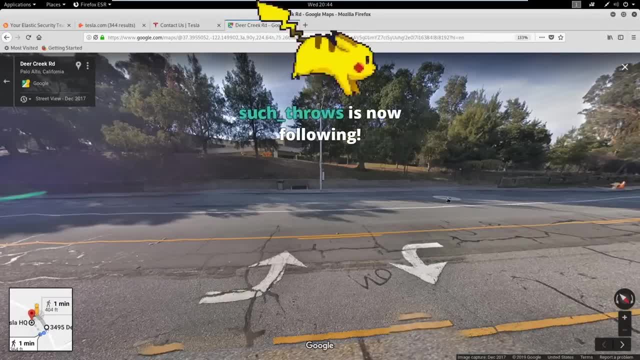 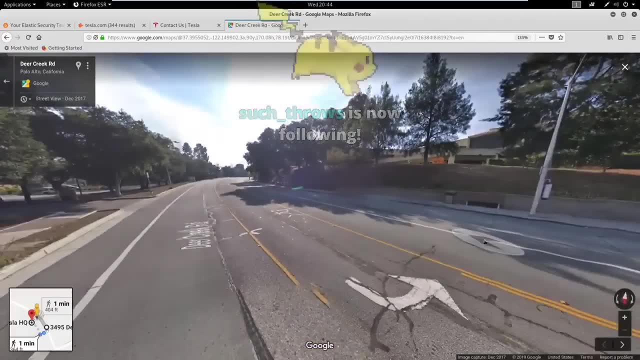 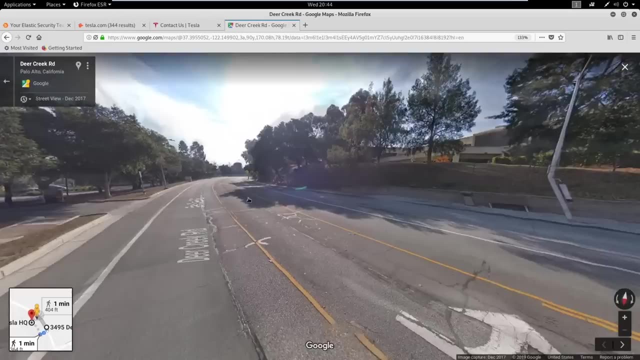 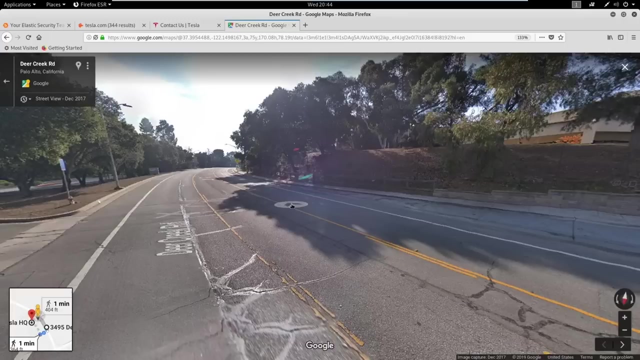 what are the chances they have guest wi-fi? they might. i would think they take their security pretty seriously, especially being on platforms like bug crowd or hacker one, whatever they're on um. but you know you can't just judge them and say, yeah, for sure that they're going to be safe, but all right. 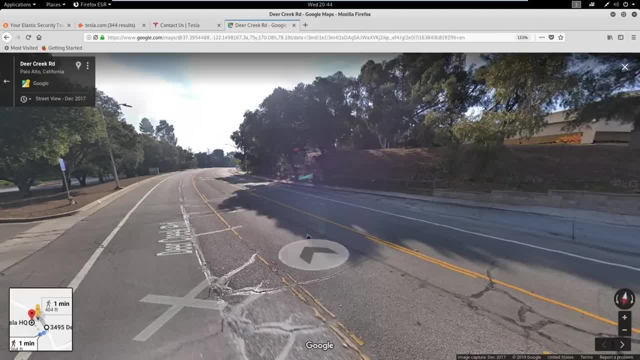 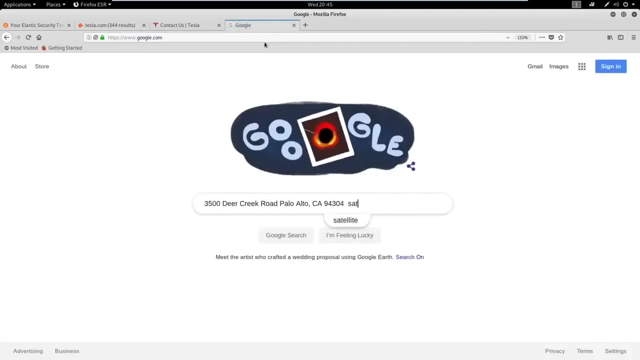 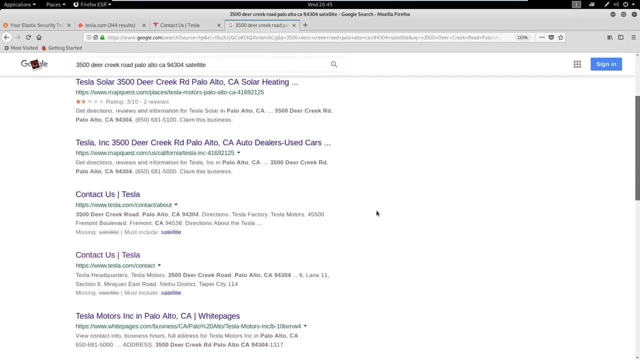 that is true. date timestamp might be important here. this is from december 2017, so what has happened in two years so we could take satellite images? we can try this right and if we put this address in and we say satellite, let's see. i don't know all the good sites, i just want to make sure that i have all the good sites. 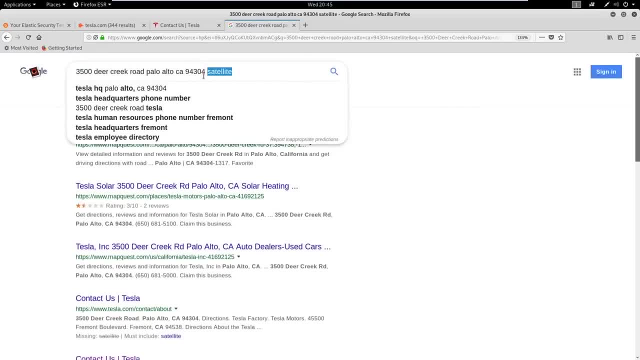 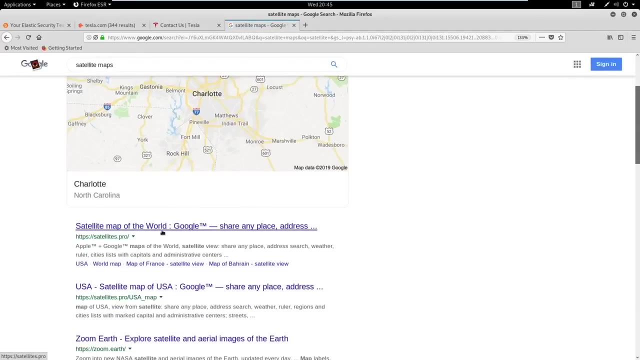 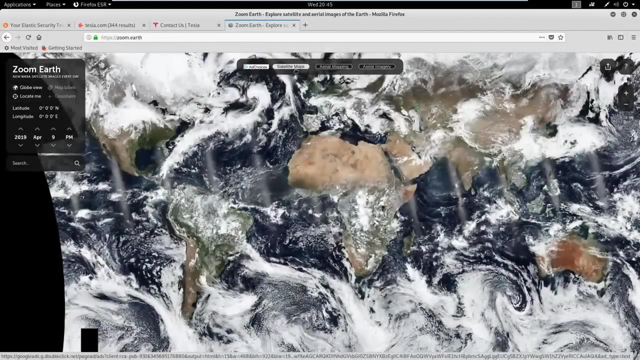 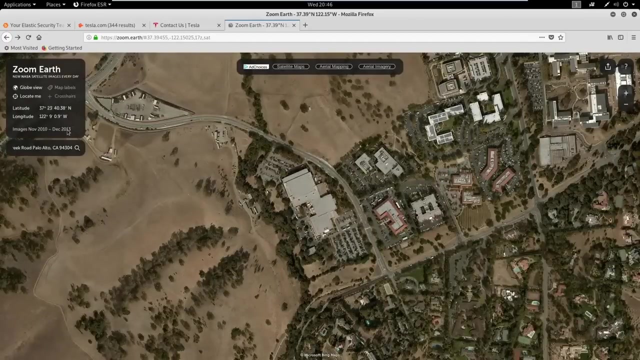 let's see. i don't know all the good sites, i just want to make sure that i have all the good sites. have to come, come across them. if you know a good site, let me know. do See, these images are from November 10th to December 2013, and this is Microsoft Bing. 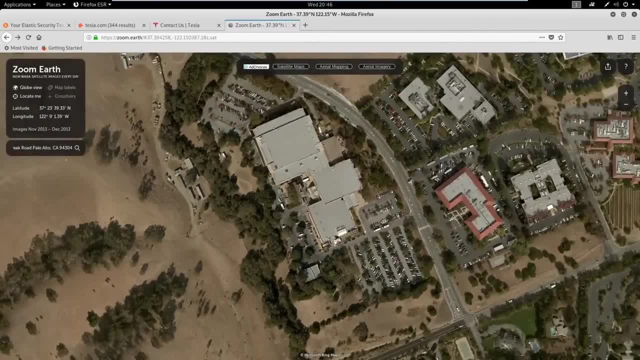 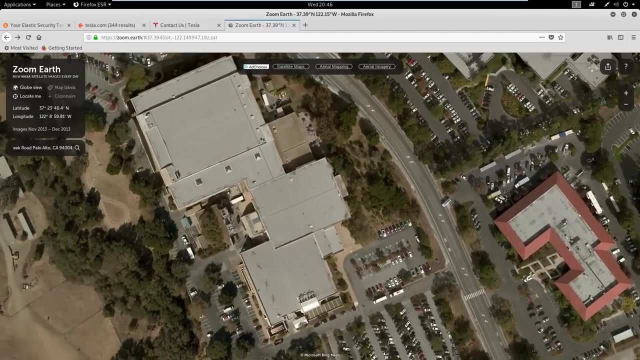 So, yeah, their security presence could have increased, maybe even likely did increase, Right. so Tesla was more coming around, not as popular at that time. So things to think about, But we'll move on. We won't stay too long with satellite images because we're not doing a physical test of Tesla. 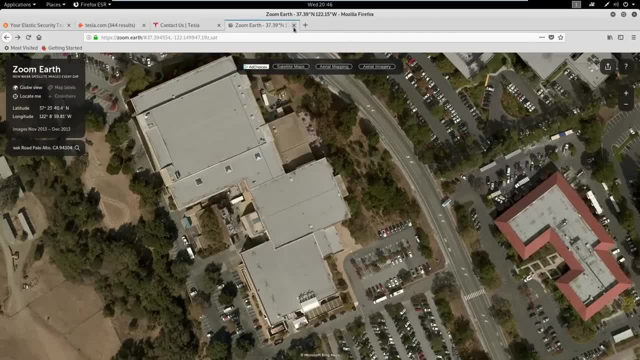 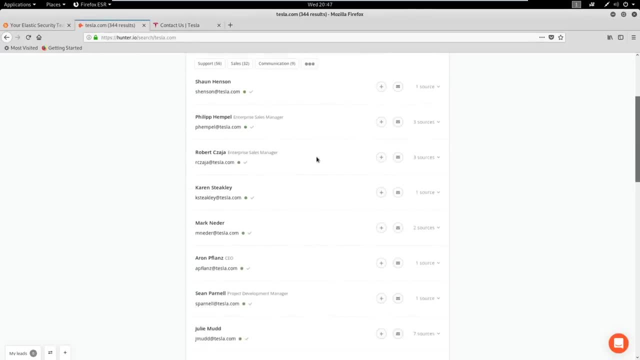 So we could go back to, let's say, people And let's just pick a name out of here. Let's pick this guy, He's got a kind of unique name. Or this Stephanie has a McCandles or McCandless. 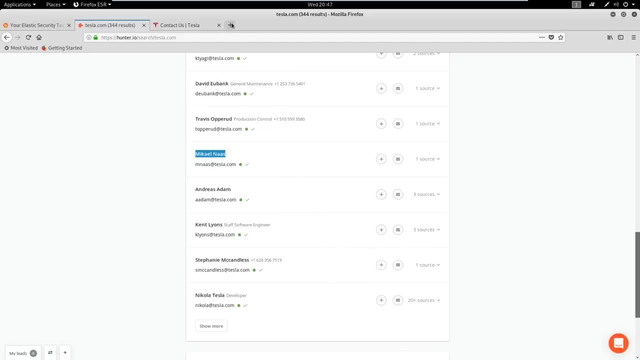 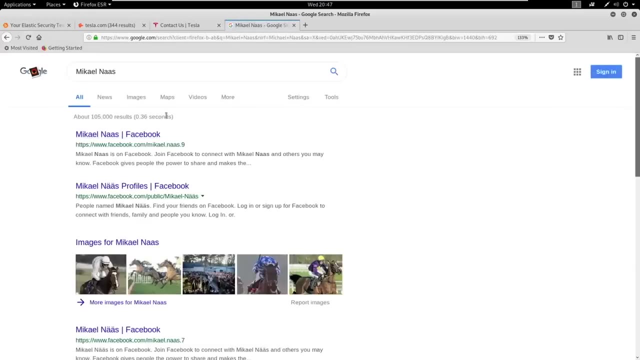 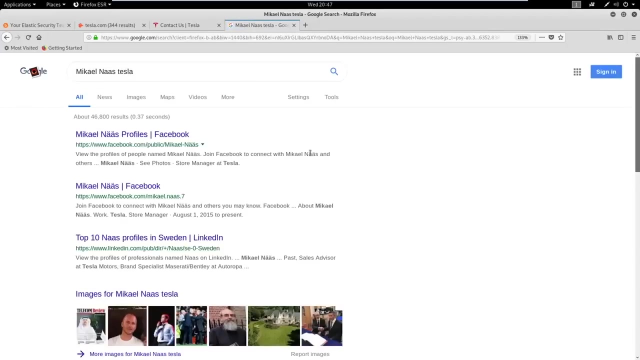 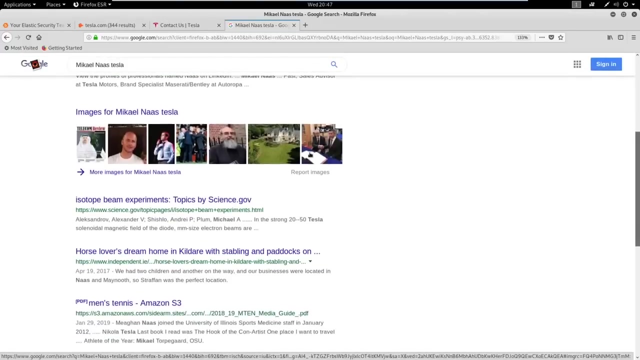 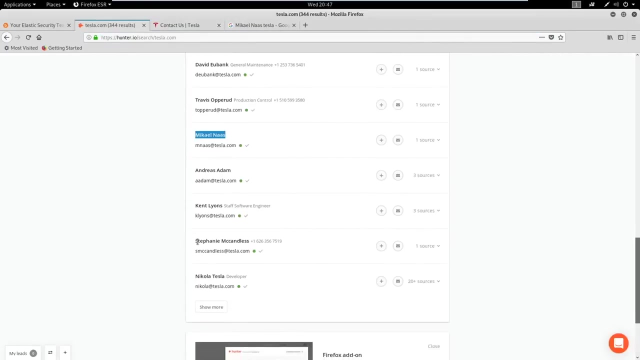 I don't know. I like McCandles, We could search for him. We could say: looks like this is actually more common than we thought. Let's pick a different name. Let's pick a different name: Nikola Tesla, nice, We could email that address. 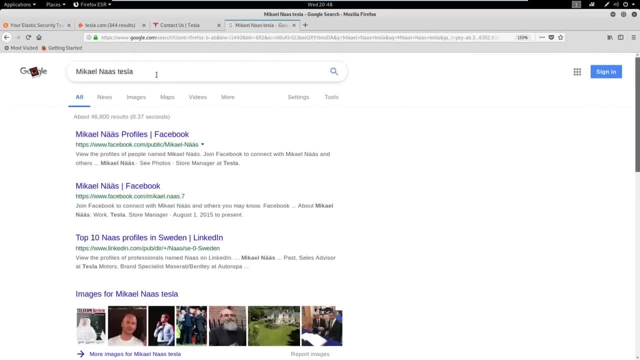 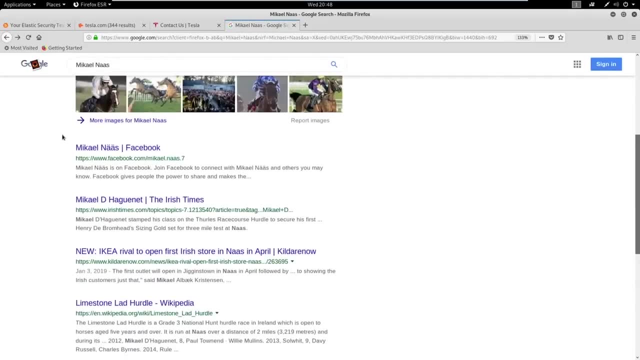 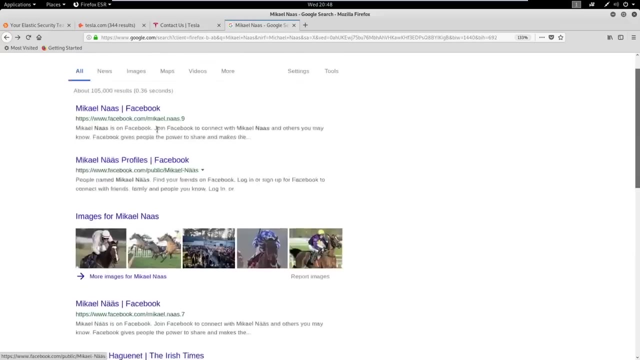 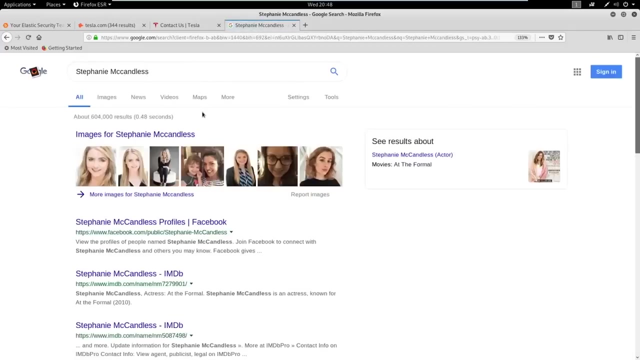 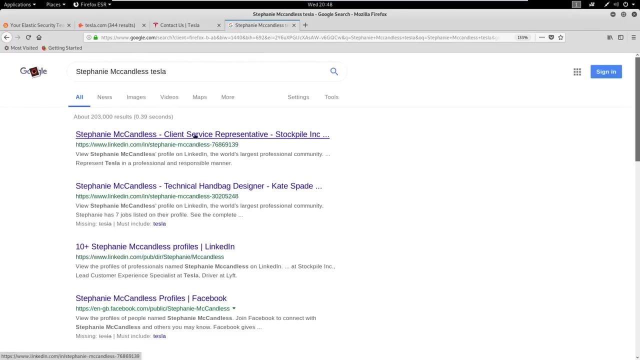 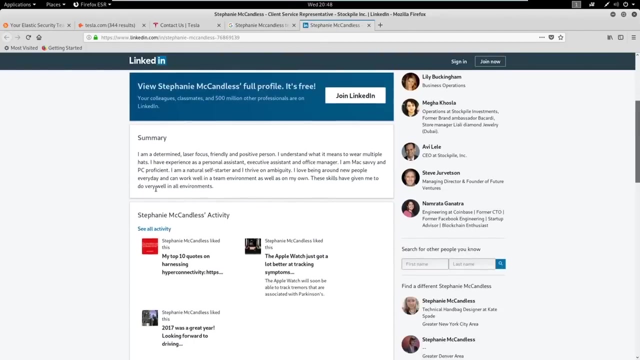 That's actually pretty funny. Was that an article about a guy stabbing? Okay, Guys, Where do you see a stabbing of a horse? Alright, so let's go ahead and search for Tesla And And Alright. Alright, Does not work at Tesla. 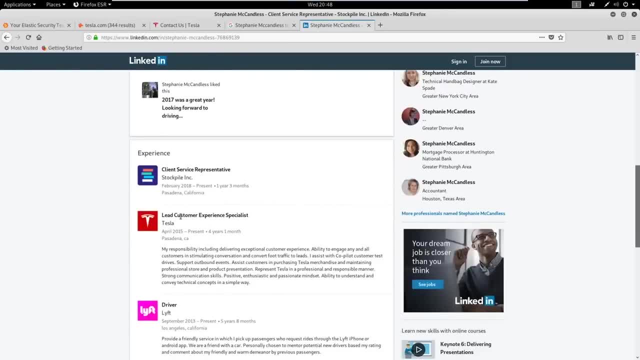 Doesn't look like Used to work at Tesla- Oh no, she still does. Lead customer experience specialist, So probably not a high target, right, but the high targets aren't the ones we're always going to be after either, So we might be able to find some information um from someone like her If we look at her um. 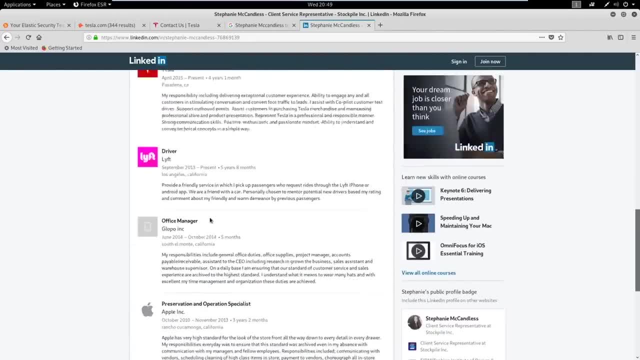 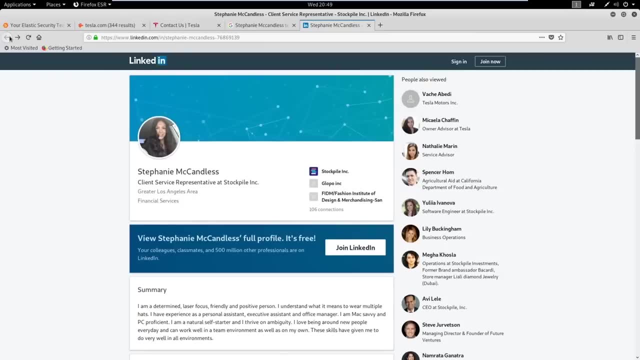 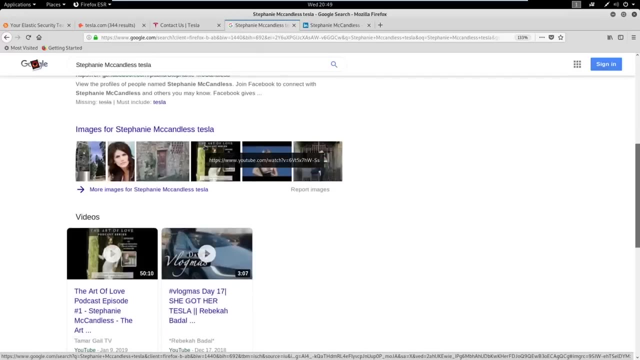 if we look at like her Twitter or her Facebook or something along those lines, and she looks completely different, What are the chances, man, that she has the same name as an actress or whoever else with that unique? Oh, we're going to get into some Google hacking. 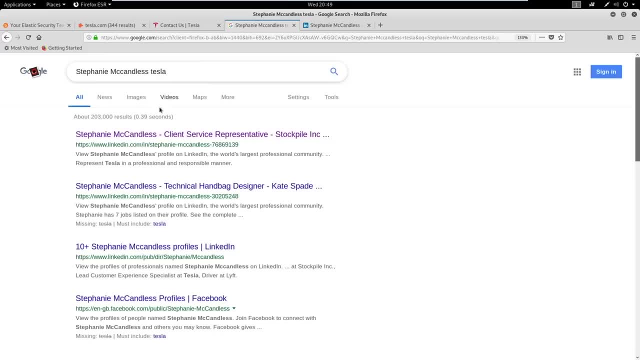 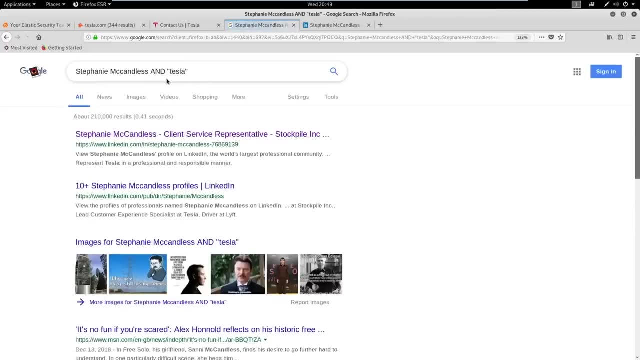 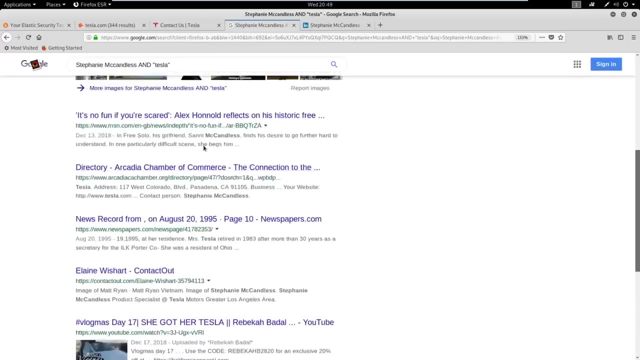 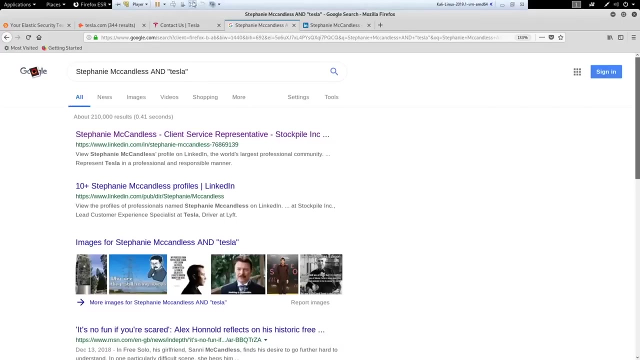 Well, she's a client service representative. Let's not judge her income. We won't spend too much time, uh, too much time on people either. So if you guys find anything interesting in terms of people, let me know. There's a lot more tools that we need to go. 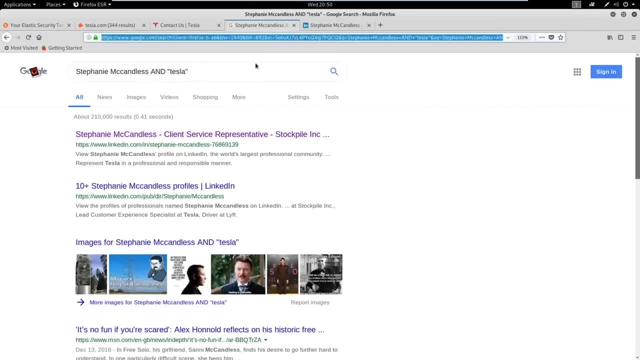 through before the night is over, Um. but while we're on the topic of of this Google foo or Google hacking, there's a bunch which most of you are probably very familiar with, Um. but let's say, for example, we want to search for Tesla. 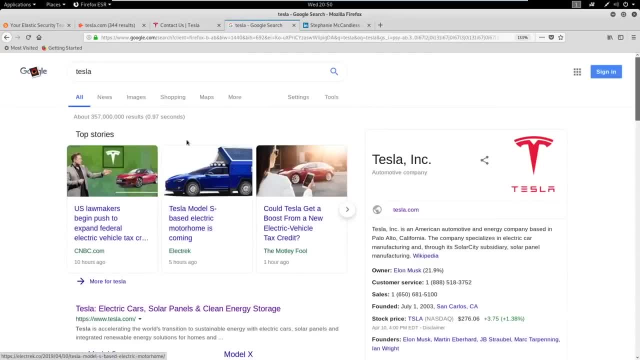 Uh, and we say, okay, well, we found teslacom, Let's search teslacom. But let's say we want to find um. well, let's say we want to find information on that site and only the site of. 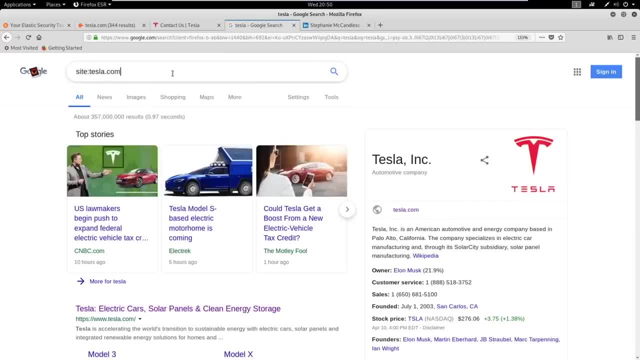 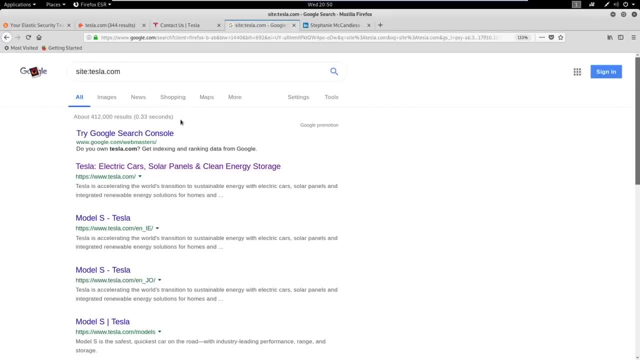 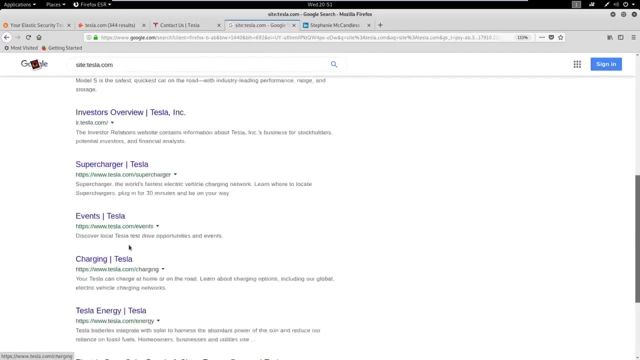 teslacom, right, We could say site teslacom, Okay. And then we come in here and we see a lot of wwwteslacom and we can get all these directories that are in here. Um, but what if we want to see maybe some sort of sub directories? 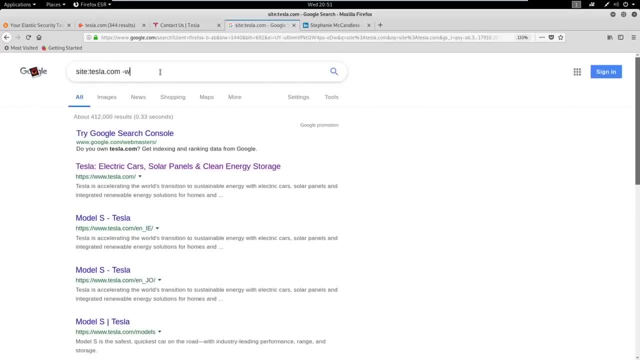 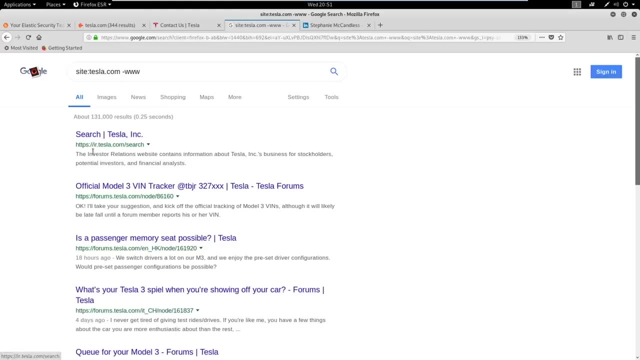 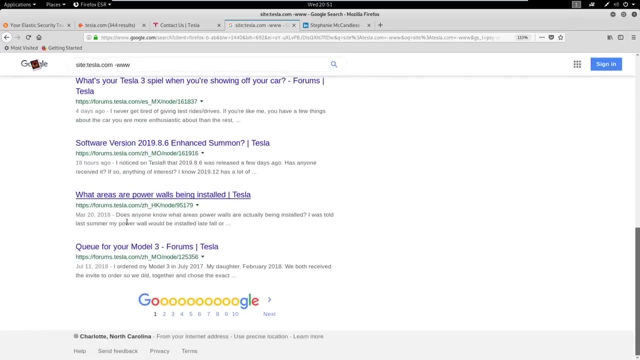 Uh, we don't want to see any of the www. We could take out the www with the minus www, And now we get other sub directories, right, We get irteslacom, Formsteslacom, A lot of forms, And we could start minimizing this. Maybe we don't want to. 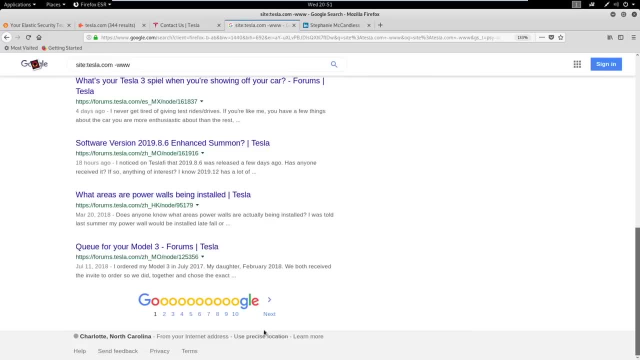 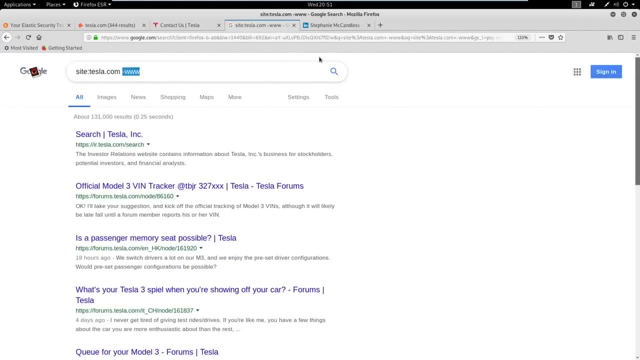 see forms. We can take out formsteslacom. Um, so we can. we can do things like this. We can also look for interesting docs, right? So we could say file type PDF and only look for PDFs that were put out. 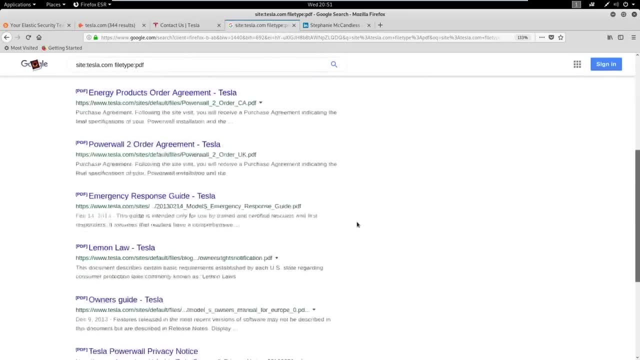 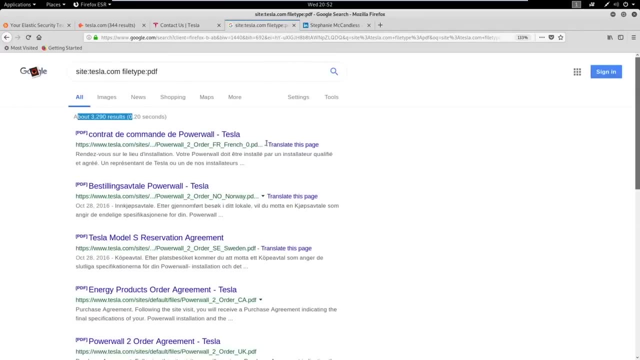 Um, sometimes you get interesting information that's left behind. How many PDFs does Tesla have? Tesla has 3,290 PDFs, Um, but who knows what they may have accidentally put on there, right? Uh say, for example, you might see financial statements you weren't supposed to. 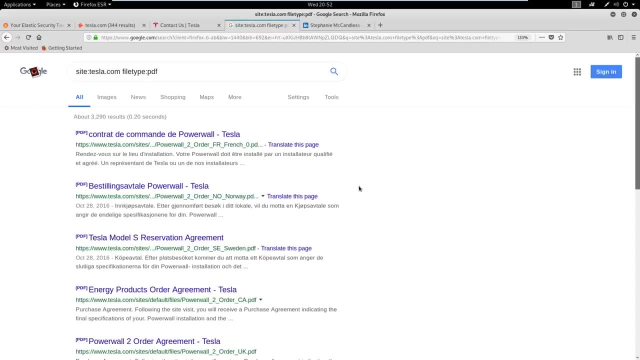 or client information you weren't supposed to, or some sort of sensitive information. Just as an example. uh, doc X is a good one to look at. Uh, it looks like sick in the mind just posted a pretty long file type one. That's pretty good, Um, so yeah, there's a lot of. 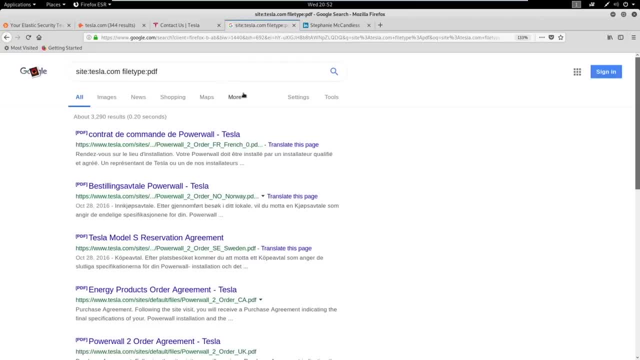 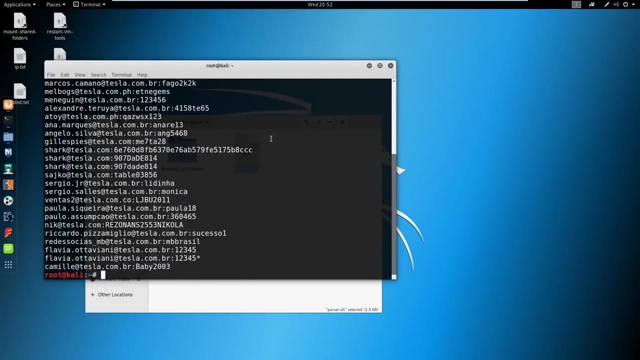 interesting file types to look for and just things to think about. Uh, other than looking for files and people, we can use other tools that are built in already. So we talked about the harvester a little bit. Uh, let's just type in the harvester like this: 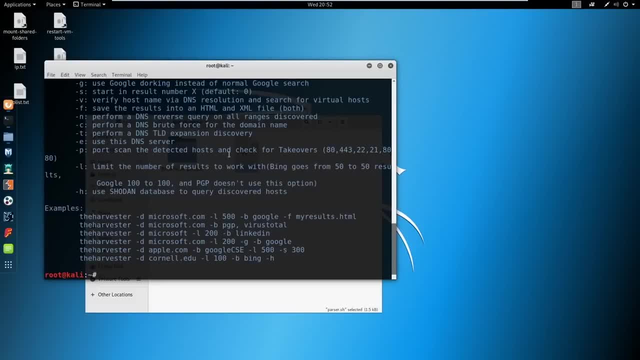 Now, if you run it by default, it's going to want API keys, uh, which we don't have at the moment. So we're going to do is we're going to fill out the old fashioned way, or, if you actually run it with, uh, a dash all, which is an option. 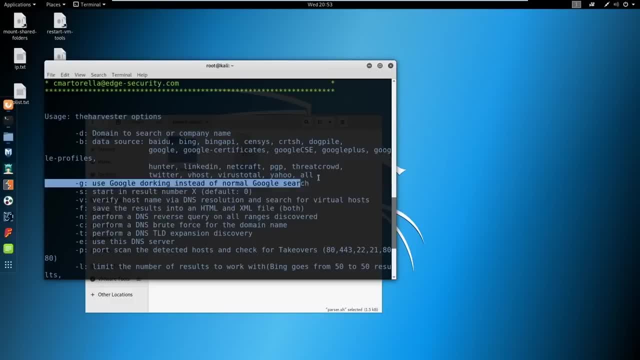 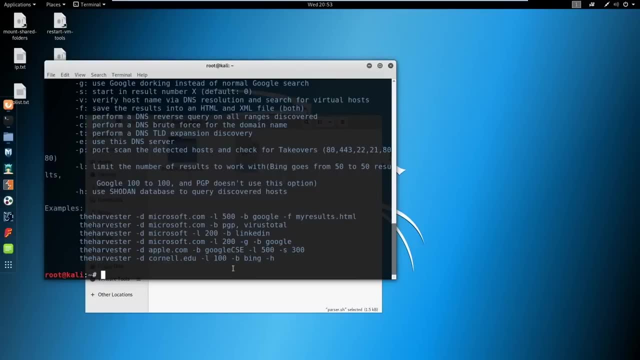 here, then it's going to want the- uh, the hunterio, these ones, the API key to actually search. So let's just take one of the examples that are here. Let's say we want to search the harvester and we want to do a domain of teslacom. 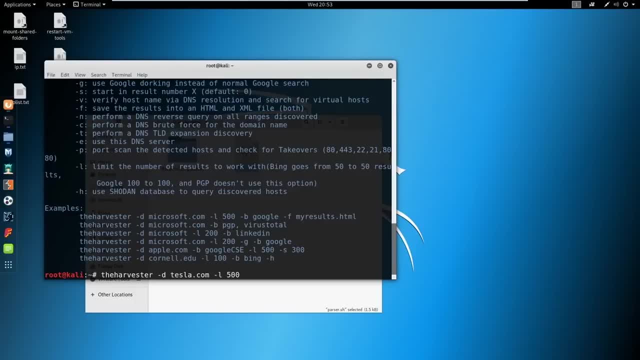 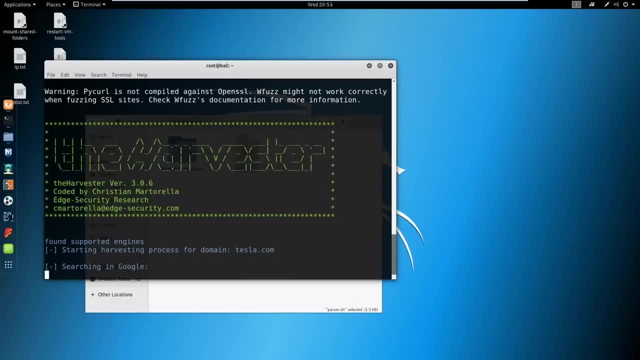 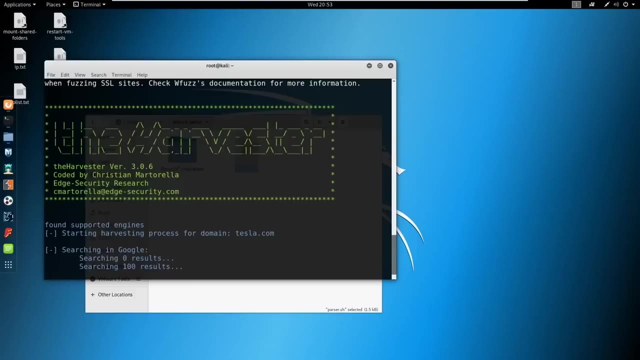 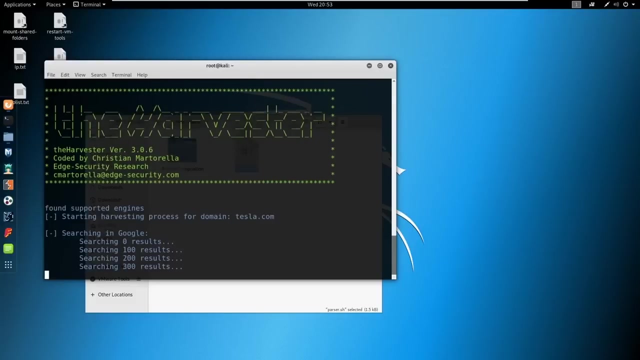 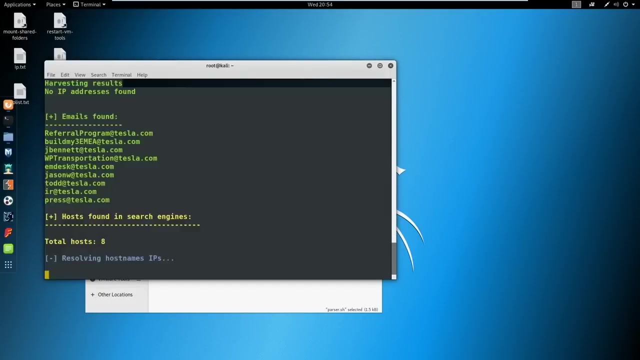 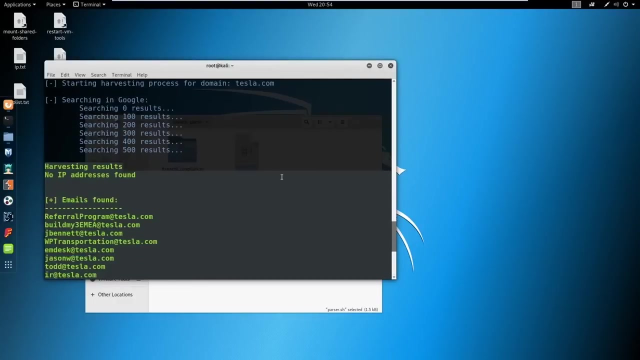 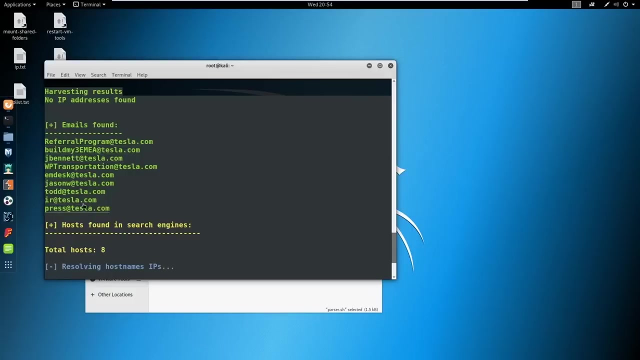 We want a length of 500 searches through Google And let's just see what it pulls up. This'll take a minute. Hey, Nanjo, how's it going? Okay, so it looked through it. It found some emails um potential targets here, just gathering information. 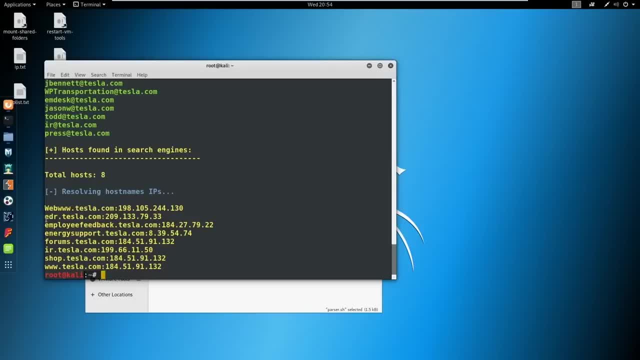 It also found some web addresses. Look at this. They found some more subdomains: edrteslacom, employeefeedbackteslacom. We see the forms that we found: IR shop, energy support. Um, we might find something again interesting in these subdomains, right? 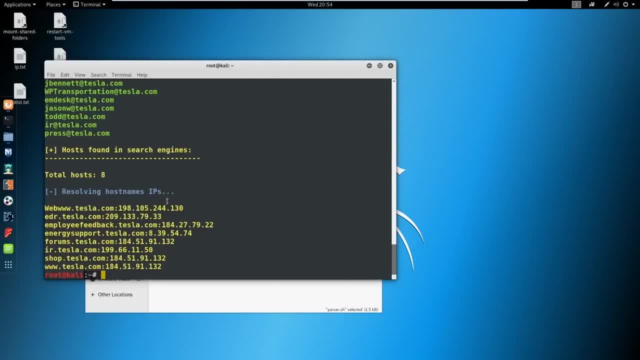 Like a devteslacom, That might be interesting. Um, these types of environments, uh, we might find an interesting email like help desk or something you know that might be interesting to us at some point. Uh, it's all about the information gathering at this point, as much information that we can gather. 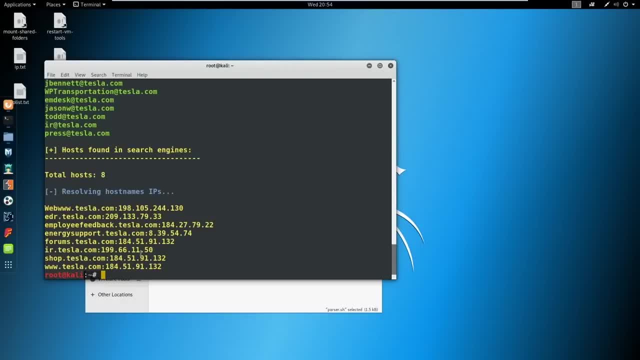 Uh, to perform our attack. Now, when it comes to doing penetration testing, which is more of what this course, uh, revolves around, we're not going to be doing a ton of this in our day-to-day work. Uh, the the things I showed you when it came to searching through breach password lists, that's definitely something you're you're going to do in a day-to-day. 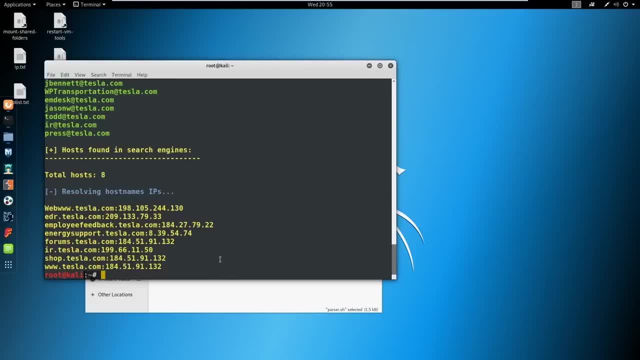 Uh, if you're doing social engineering engagements, depending on where you go, if you're doing network pen testing, you're probably not going to be touching this kind of stuff, Um. but if you do move into social engineering engagements, you go to a true red team. 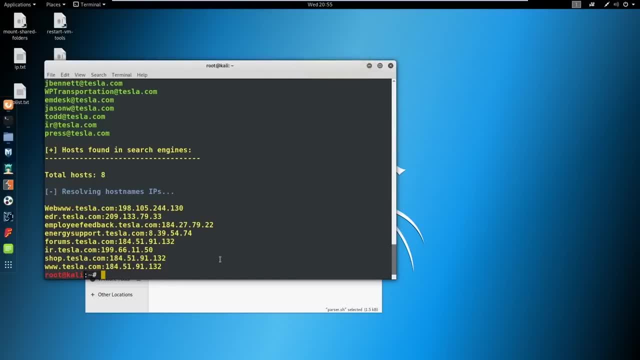 Uh, this is where information gathering and mapping out and stuff becomes important. Uh, so the things that I'm showing you, the things you're learning, you may not see again for a long time, Um, but it's still useful information to know how to search for things. 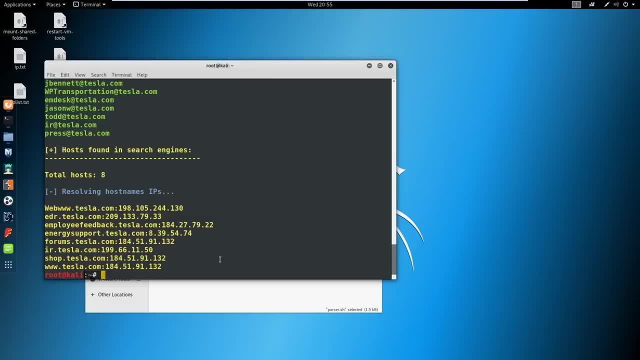 Uh, but Google is probably far and away your best friend, but there are definitely tools built like this out there to help you sort through these things Um. another one that we've touched on and talked about is: have I been pwned? 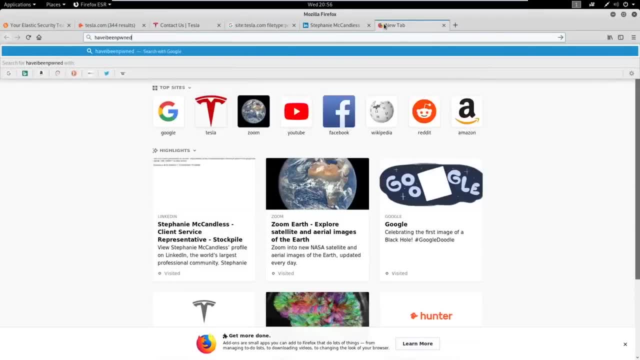 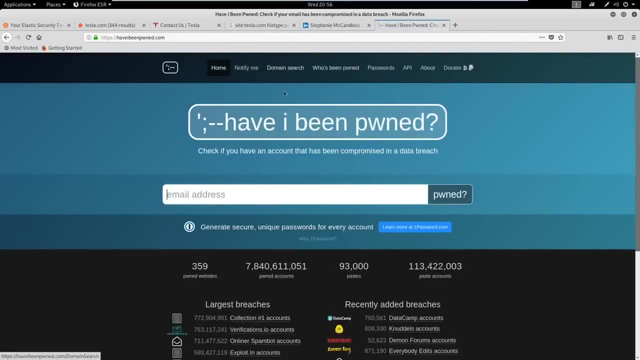 Right Say, have I been pwned like this? You haven't heard about this. This is a good thing to sign up for, Uh. you can search your email address in here to see if you have been pwned, uh, and what breaches you've been a part of. 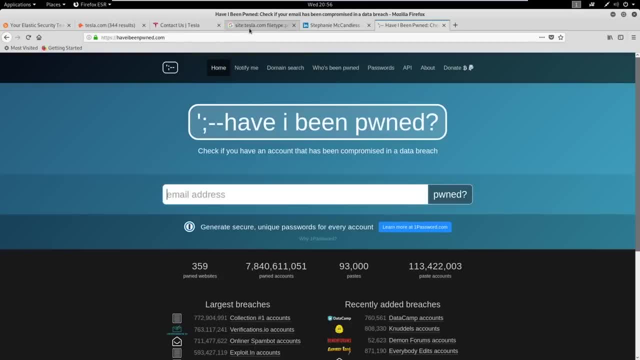 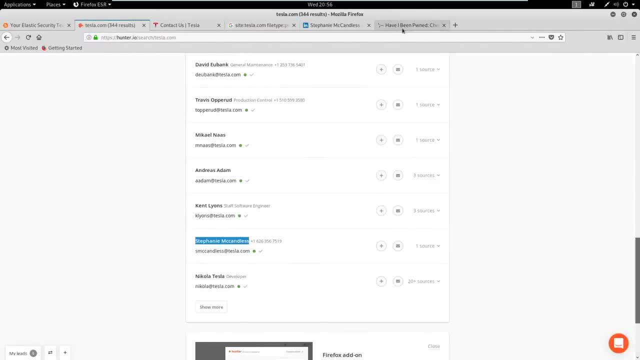 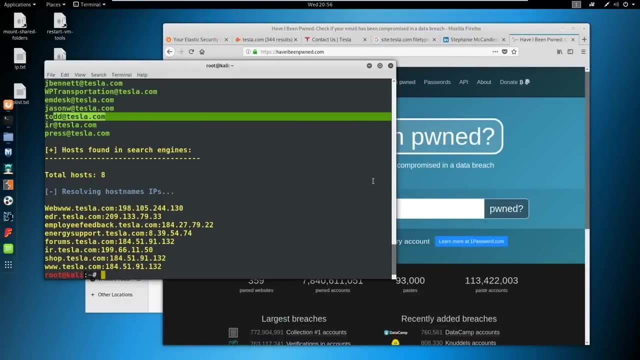 Now there are tools that are out there that will allow us to search through Have I been pwned? list To see, Yeah, Um, if the user that we search has been pwned. but let's take, for example, um, one of the emails that we just found: we've got Todd at teslacom. 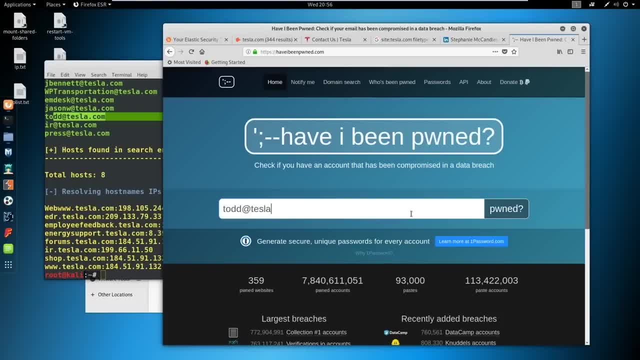 Let's just try him. This is just for conceptual theory. This isn't for Hey, this is the best uh method. Obviously, if we searched every single Tesla address like this, it would take forever. That's why there's tools out there. 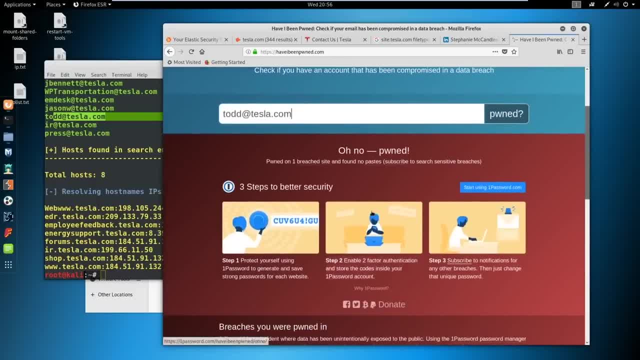 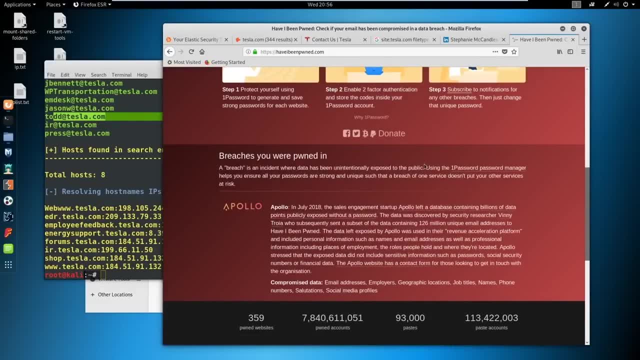 Oh no, Todd has been pwned. Todd was pwned in July of 2018 in the Apollo breach. That was quick, wasn't it? So it looks like he has some information out there. Now, if we were to go find an updated list, or if somebody has his hash and cracked his hash and updates like those clear text password lists- um then, 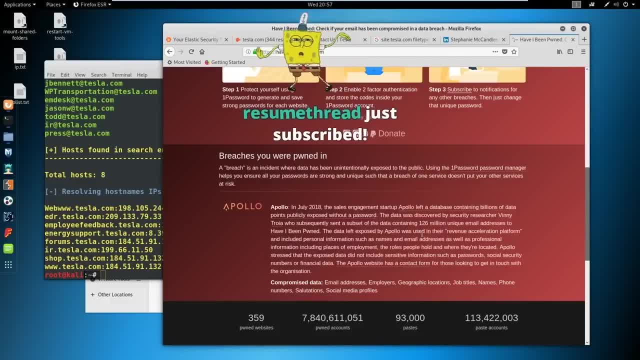 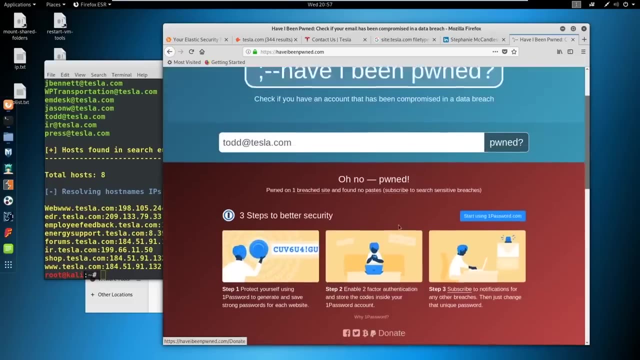 This becomes dangerous, right? So uh wasn't expecting to find that, but that's a great first example to grab and see, And this is pretty recent. Um, thank you for the sub resume thread. I appreciate that. Uh, so things like this critical to look for, right. 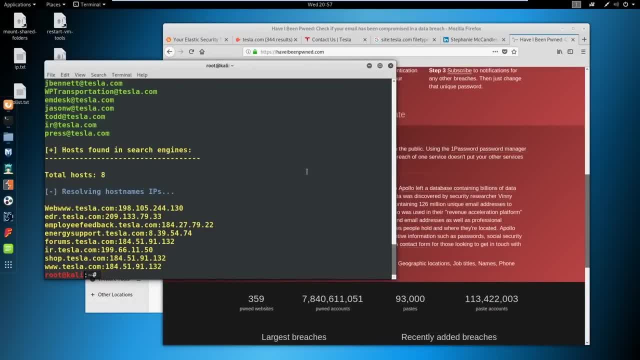 Hey, Nate dog, How's it going, man? So there's a tool that kind of does this for us, called Bluto, So I've had some issues getting it to work. on this, The machine, um, I'm going to show you how to install it. 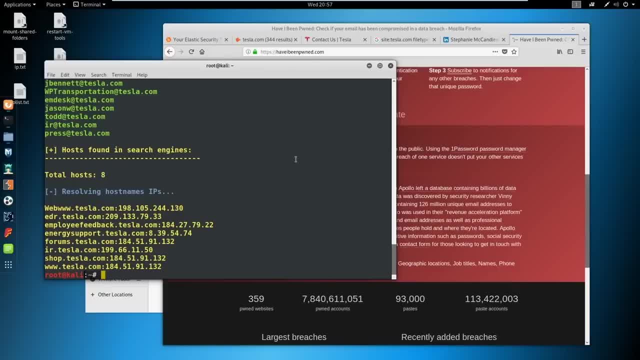 Maybe you'll have better luck than I do. And what we're going to do and what it does is it looks through- have I been pwned information? It does some active recon. Um, it does try to do like zone transfers, things like that, where it's trying to get more information. 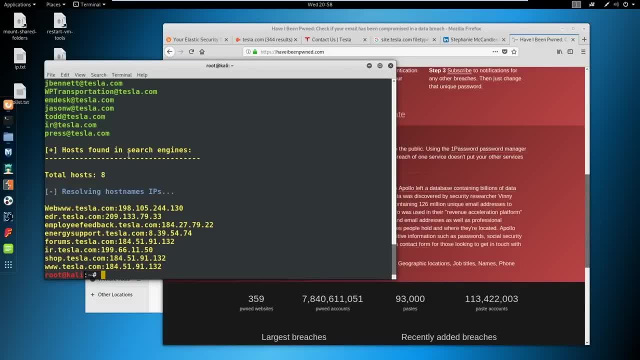 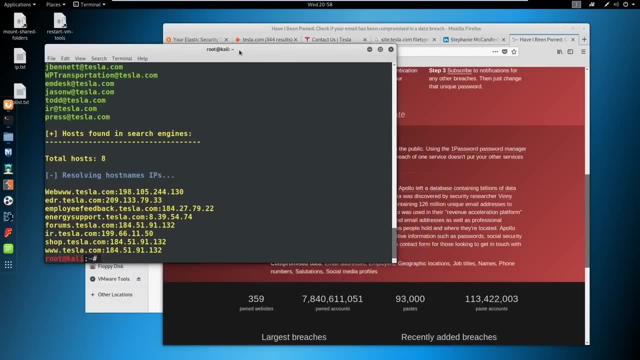 Uh, so be aware that we are actually hitting the site There will do some brute forcing as well. So be aware of that. Um, because Tesla is on the bug bounty Program, I'm not concerned about it. but don't just up and run this against any site because, uh, you will generate some noise. 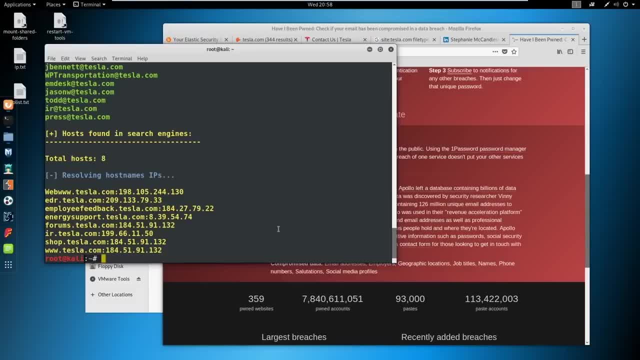 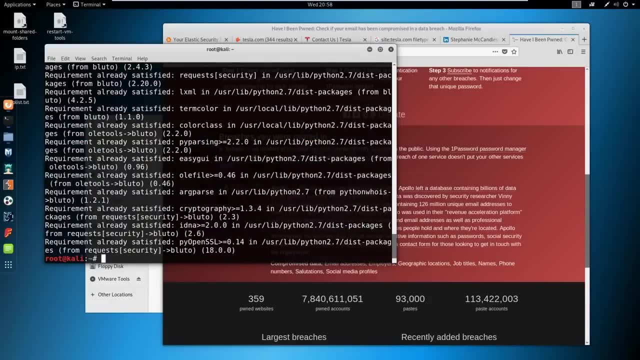 Uh, so if you want to install Bluto, the command is just pip- install Bluto. like this: It is already known by pip, mine is already installed. Um, so when I went to run it yesterday I was testing it out, because I don't have it. 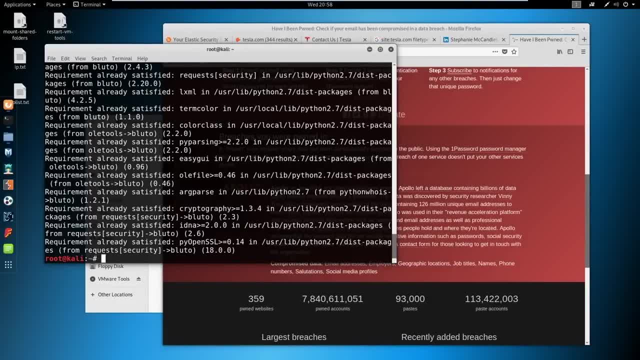 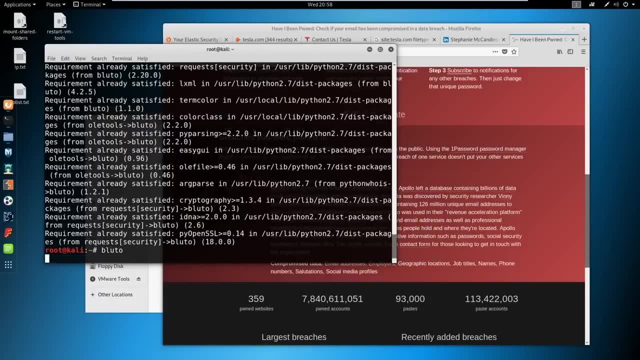 This is my student computer. This is the one I use for you, Guys. Um, when I went to test it out it was broken. So if we type in Bluto, let's see. I did fix it. Let me control C. 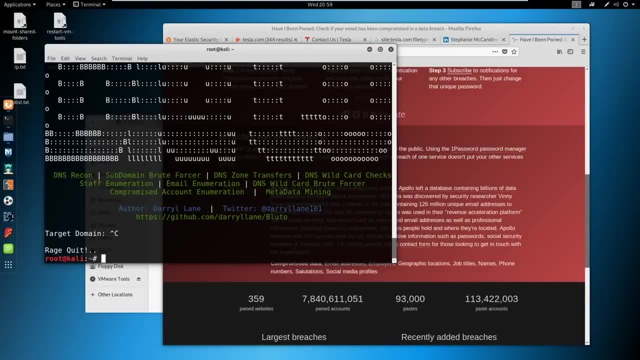 Okay, So if yours, when you type in Bluto, does not work, it may something say something along the lines of an error on the module named all file. Oh, L E, F, I, L E. Uh, you should be able to fix this through the lessons that we have had in the last few weeks. 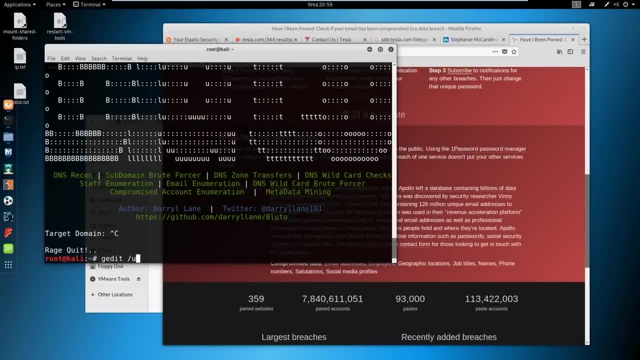 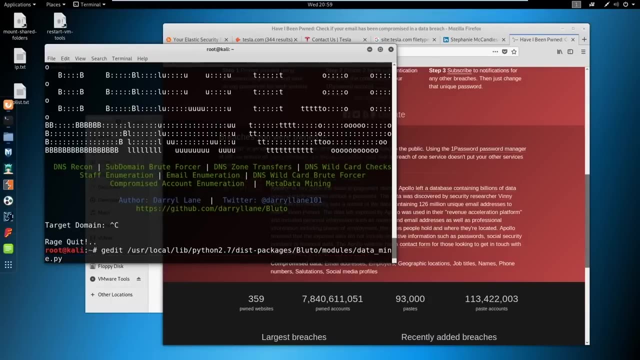 But If you look at the file that was of issue, which I'll type out for you guys in case you're watching this later or following along now, this is the directory And we're going to edit this data. mine dot pie. 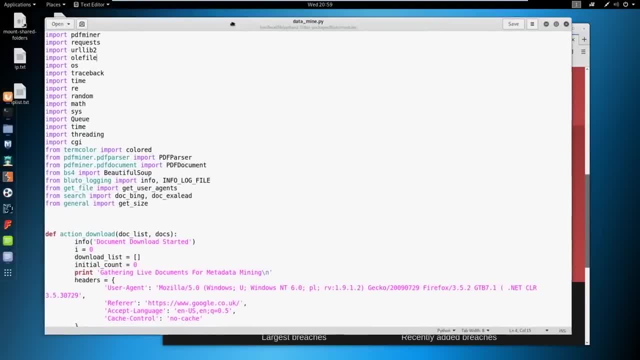 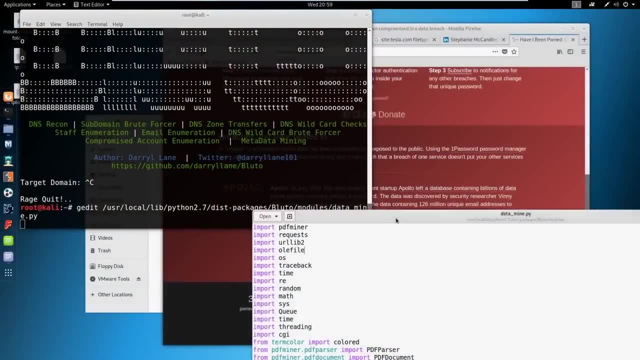 And I'll bring this up for you guys. I'll let you guys look at it for a minute. So you see this old file and here's the directory. So originally it had something in here where it was importing- um, it was importing something else as old file. 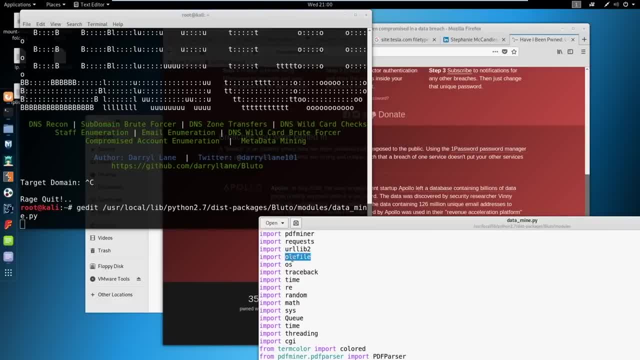 Basically, we don't need that. We can just straight up: import old file Oh L E Why? However, you say it, Um, and it'll be fine. So make this change to whatever the import originally was, to this import, and it will be fine, uh, and start functioning. 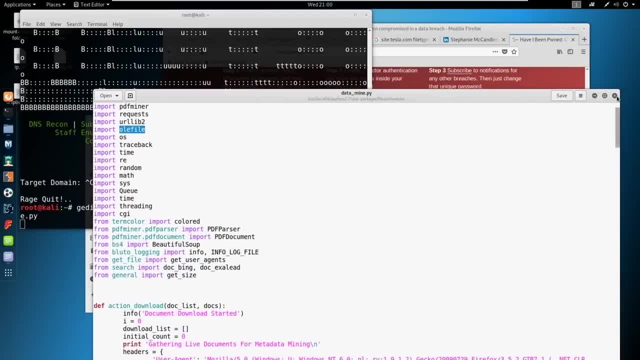 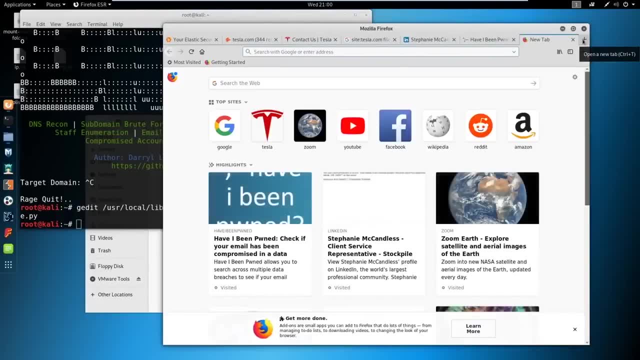 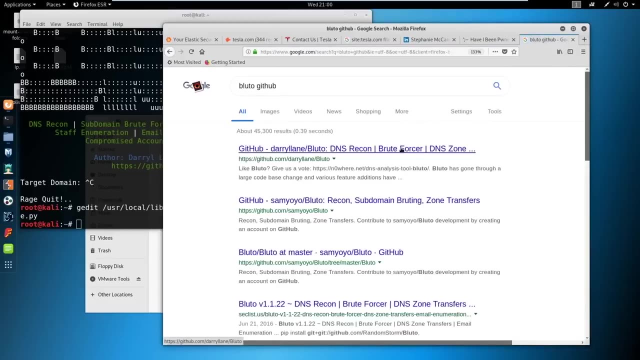 I just make sure you make that little notation there And then, once you do that, let's also go and check out the Bludo GitHub real quick. So if we say Bludo GitHub and it looks like there's actually two, which is interesting. 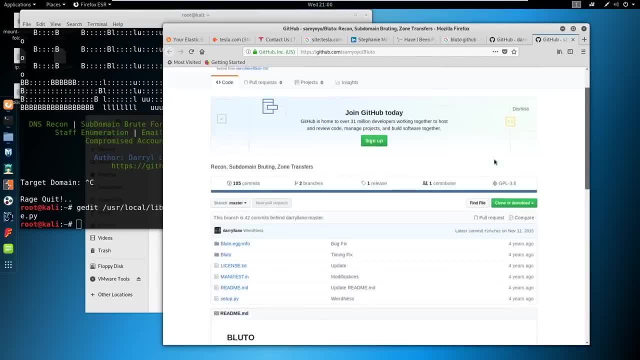 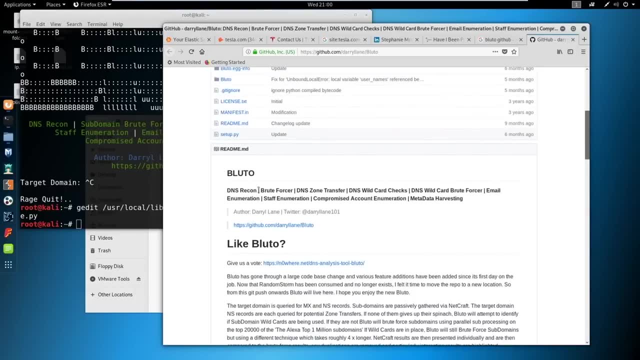 I didn't know what the difference is six months ago. four years ago, All right. Well, six months ago it is right. Okay, So it's a DNS recon, brute forcer, DNS zone transfer, wildcard checks, all kinds of stuff, right? 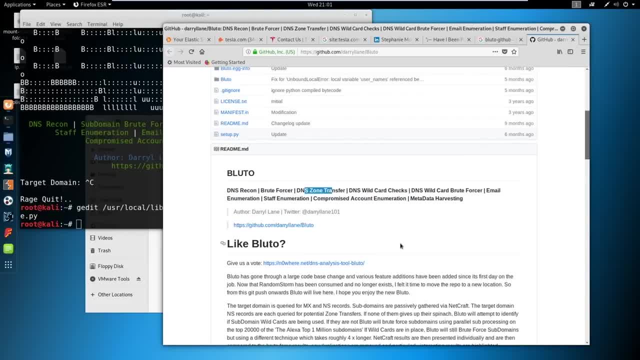 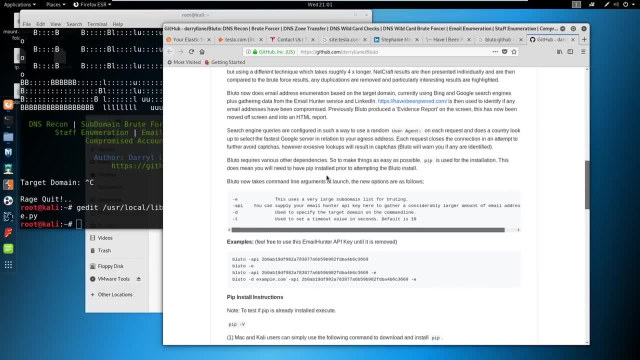 It does do active work- brute forcing, zone transfer. So make sure that you know that, as I said, going in, we come in through. here you can see what type of information you can use. Um, so here's some example. 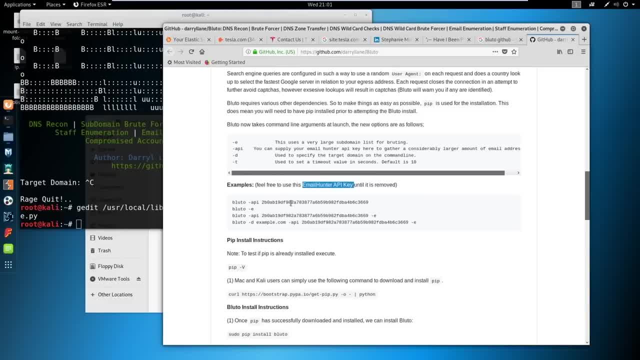 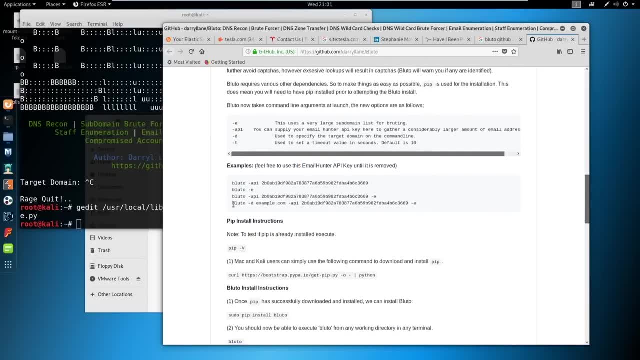 They provided an email hunter API key. until it's been removed, Who knows? I have never tried this, but you can use an API For email hunter. um, you can say blue Bludo, dash domain- also use an API. The dash E uses a very large subdomain list for brute forcing. 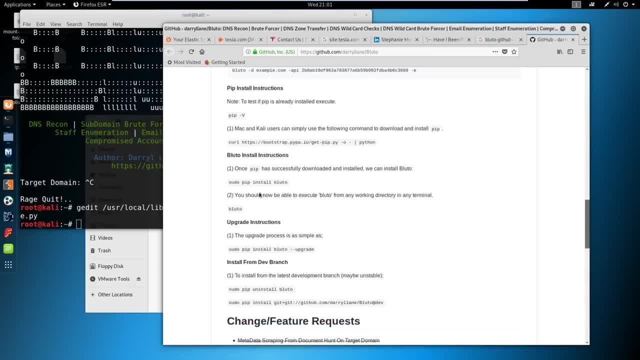 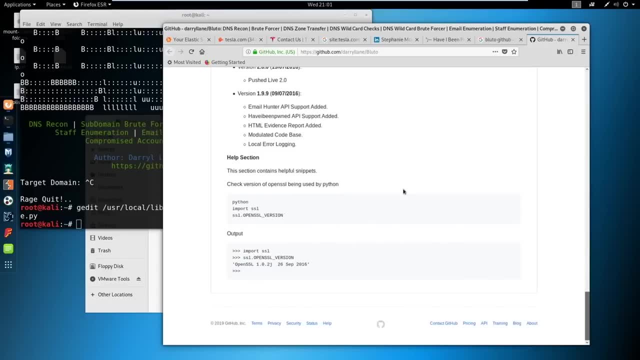 So if you want to, brute force gives you the install instructions if you need to, and then it has some change log information here. So we're going to run this. Um, it hung for me last time I ran it, but we can run it again. 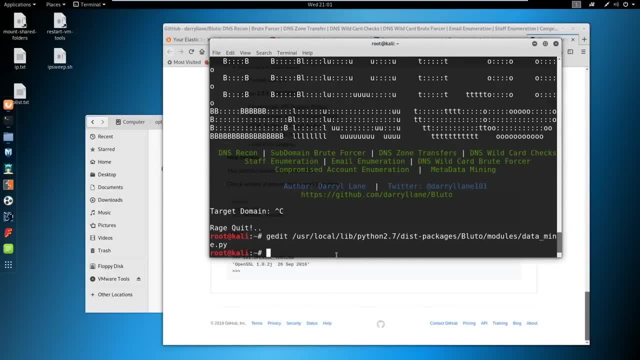 Maybe you'll have better luck. This is a useful tool If you can get it working. I don't know if it's an issue with the 2019.1 that's on right now, but it works fine on the computer that I have. 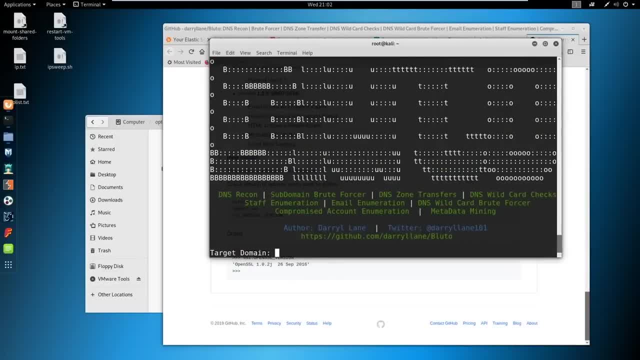 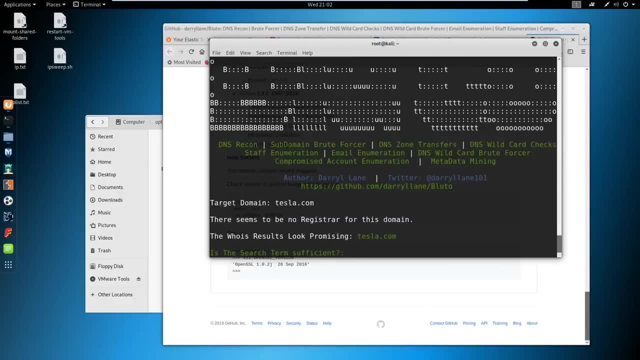 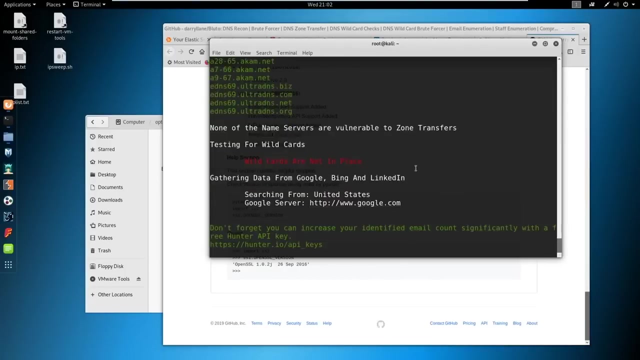 Uh, so if we just type in Bludo and we say teslacom, the points are for raffles. Davey, unless you're just trying to get rid of them all, is search term sufficient? Say yes, Okay, So some things it does for us. uh, it looks through the name servers, right? 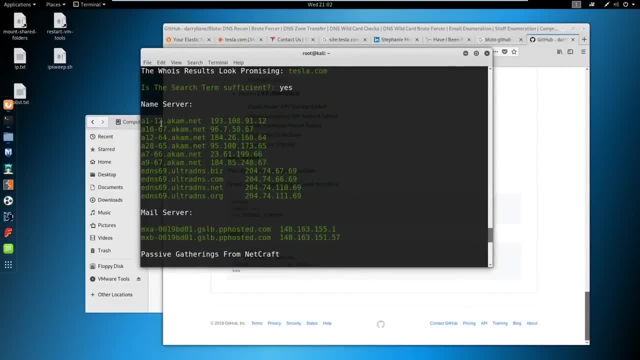 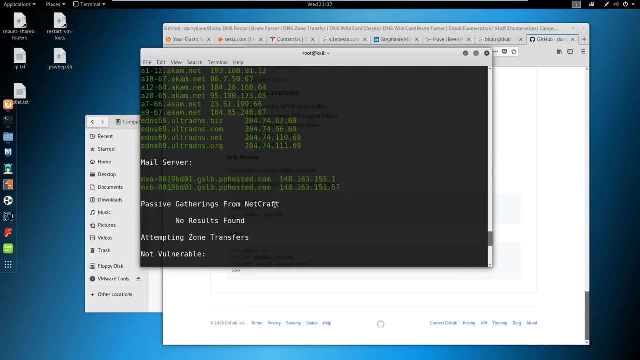 This is doing our uh DNS recon. Essentially it's finding the name servers. It's finding like an NS lookup, essentially, where it's doing the IP address scheme for the name servers. Uh, it's found the mail servers. here It goes in a net craft which I haven't shown you- net craft yet. but if you're looking for subdomains, net craft is an interesting one. 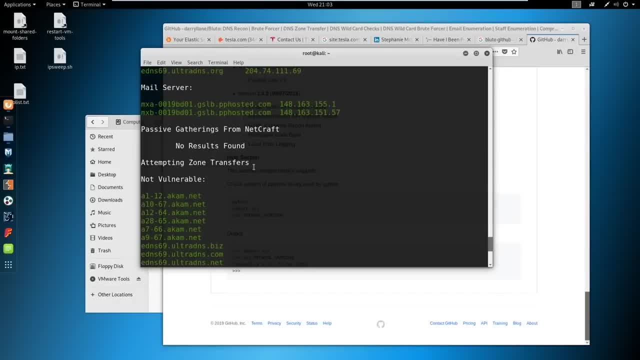 It attempts to do a zone transfer. Now, zone transfers are not common. I have never seen one out in the wild. It should still be something that you should know. Um, but basically, if you're able to do a DNS zone transfer, you are able to, uh, get a bunch of subdomains and more information. 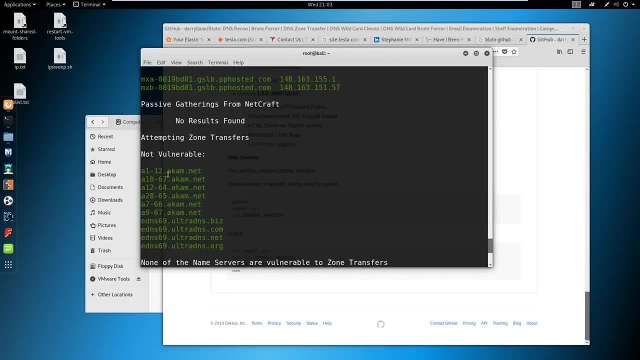 It's not. it's. It's not really an exploit, but it's kind of a vulnerability. I guess It it just allows for more information gathering for us. Um, but we don't have that here. uh, tests for wild cards. wild cards are not in place. 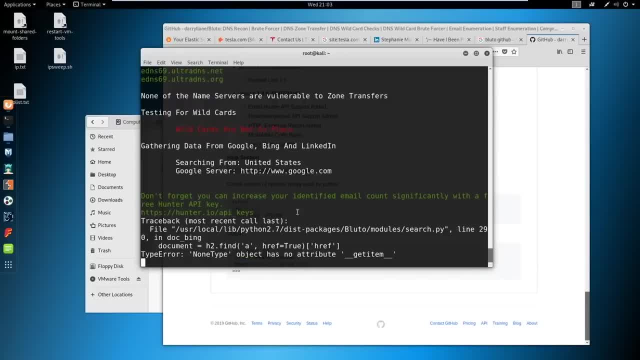 Now it's going to gather data from Google. being in LinkedIn, It looks like we're having some issues with search Dot PI. it's having an issue finding this document for being here. Um, so there may be some issues that are Are conflicting with either uh 2019.1, or there's just something in the bill that's not working correctly and we didn't supply a hunter API key. 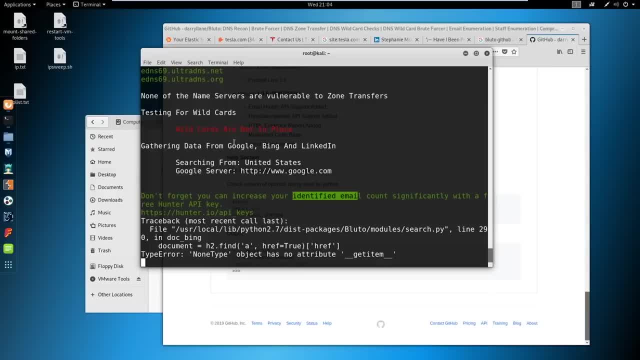 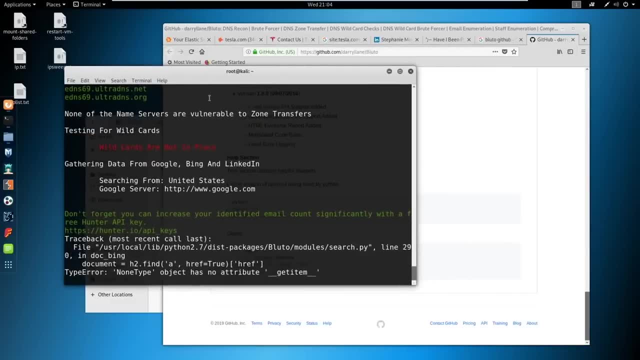 So we didn't increase our identified email account, but we can also just go search the website, like we did. Uh, so things that we can do, we'll let this run see where we get. It does download some data for us as well. 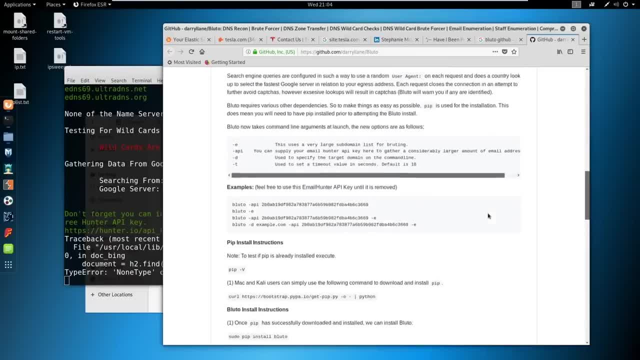 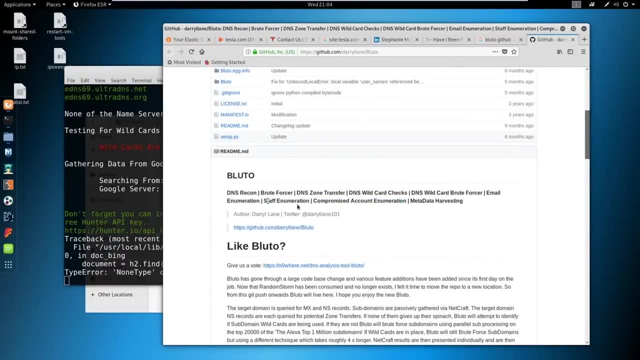 It should check through. Have I been pwned? Let's see if this one does it And I could be on an older one. But yeah, it does do. for look for compromised account enumeration, uh, staff enumeration, a lot of things. 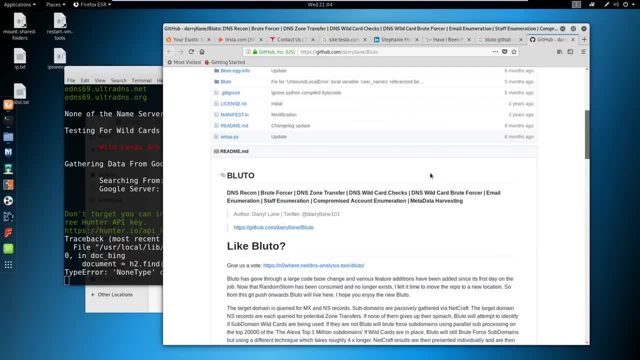 So this is a great all-in-one tool to just kind of look around and see if you can get any more information than you already have, Uh. so when it comes down to uh looking for subdomains, I listed a bunch of tools earlier like sub lister, uh, but we can also use some things like net craft, uh, or something. 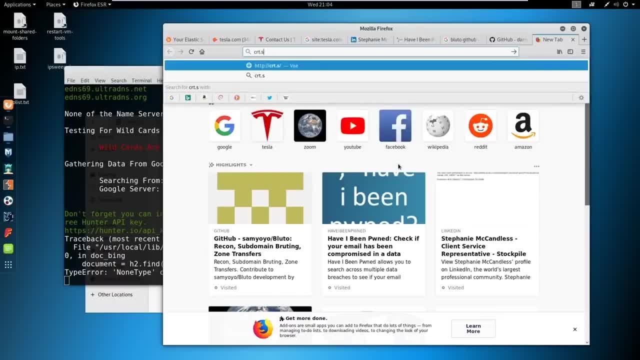 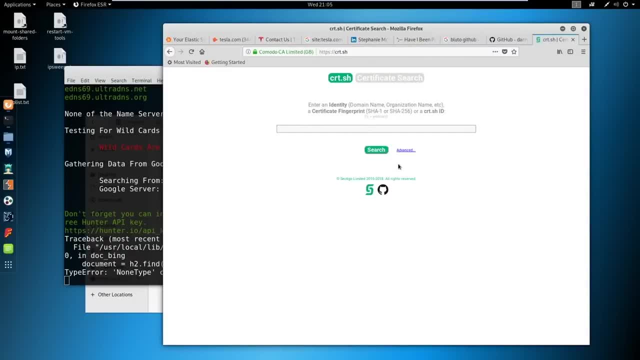 Let's look at certsh. Let's look at certsh, first crtsh. So this is the kind of the newer way to find subdomains. um is looking through these, these certificates. Um, actually, I tended to talk a local talk where somebody had built a little script to do just this and it was finding um not just subdomains, but interesting information based on those subdomains. 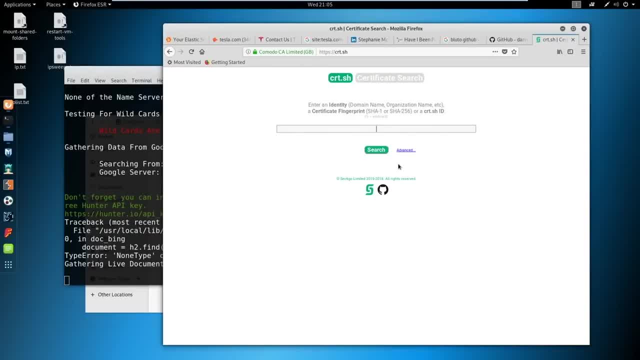 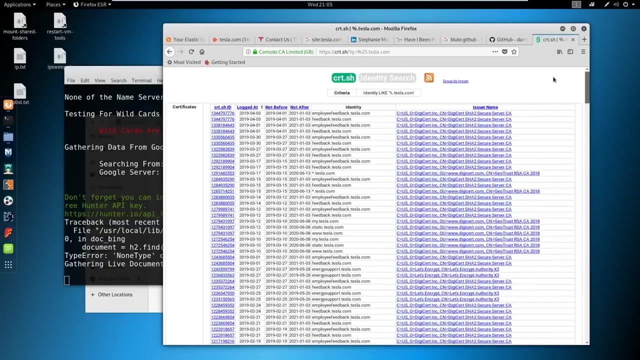 Uh, it was actually pretty cool. So here is: we're just gonna supply a wildcard, which you can see is identified as a percent over here, and we're gonna just say wildcard Tesla, calm and we're gonna hit search and if we come through here, let me increase this size. it looks. 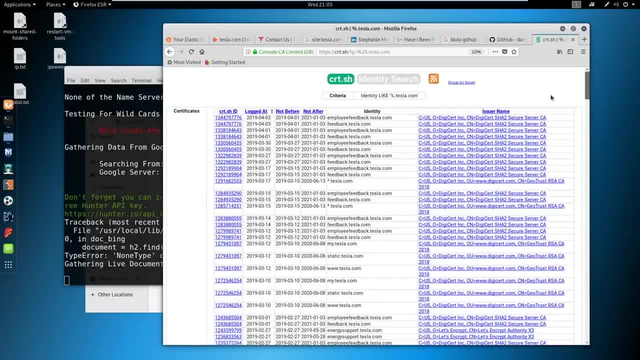 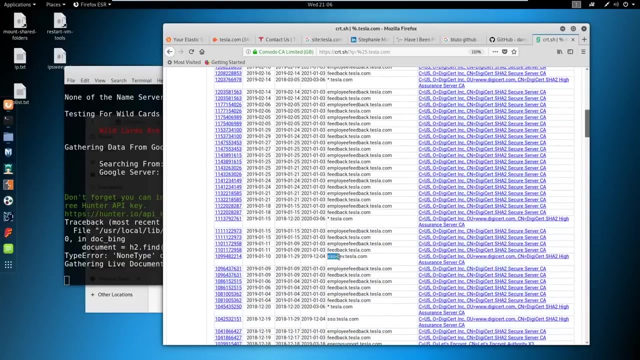 a little small on my screen through the the live stream. okay, so we get some more here. we get employee feedback: Tesla calm, feedback, Tesla calm, and you see the certificate information: right, my Tesla calm, static Tesla calm, SSO, SSO dash dev, Tesla calm, SSO Tesla calm. we can copy this one. this would be something that 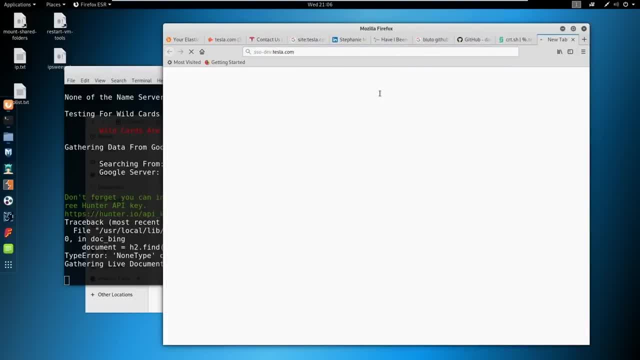 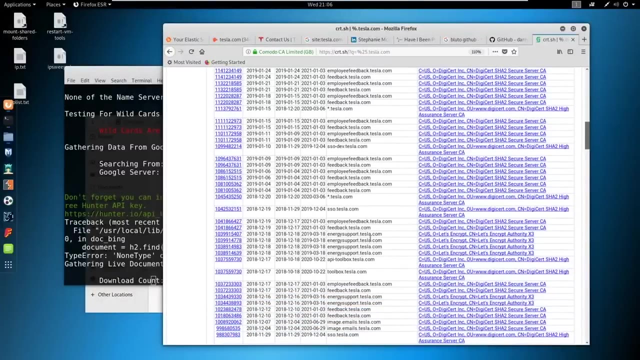 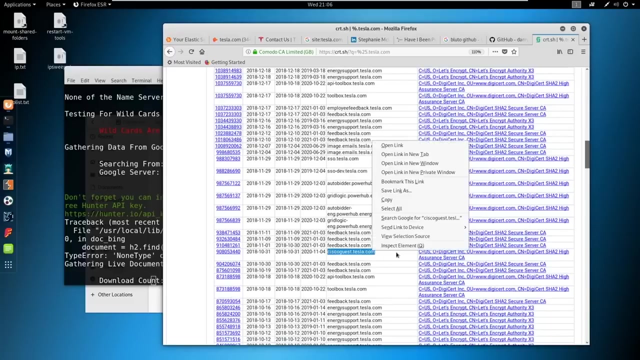 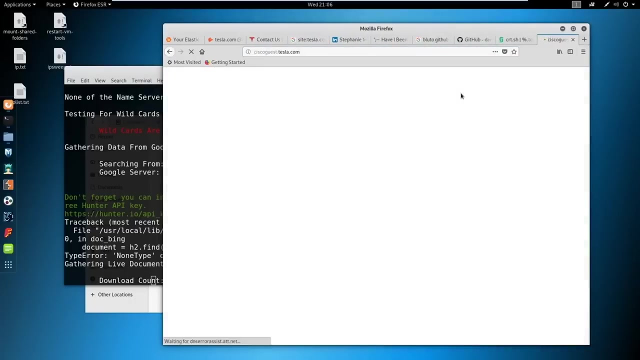 that would be interesting, right? I don't know what it is you. we may not even get access to it, since it's single sign-on. yeah, we have no connection, but it exists or did exist, right? so these are the kind of things we want to look for: image dot emails, Cisco guest Tesla calm API toolbox- try that. 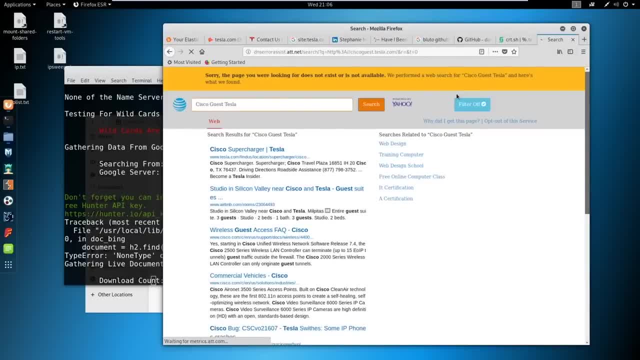 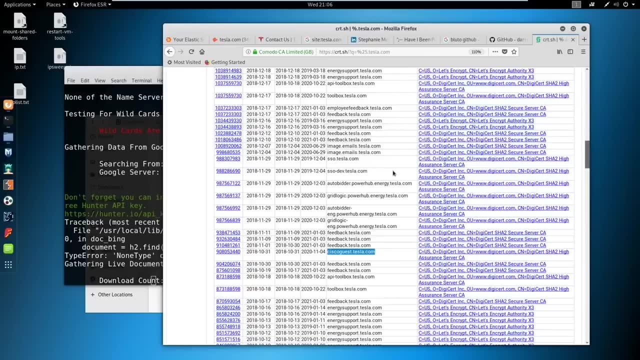 Cisco guest: nothing, we get the old AT&T search page. okay, let's see, let me take a drink real quick. my mouth is drying out. also, Cheers while we're at it. you all right, guys, heat, sir. that is probably my favorite meme, and that's all thanks to twitch. 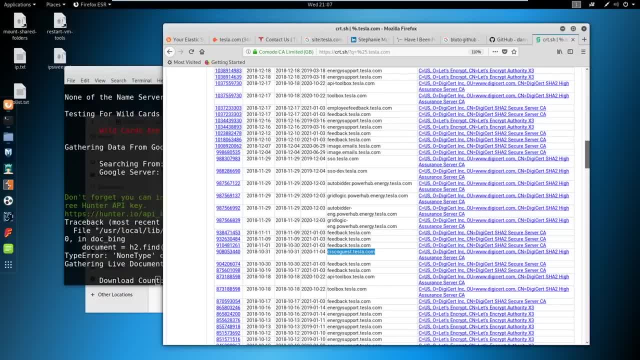 and davey davey helped create that meme and make it a thing all right. so let's talk a little bit about fingerprinting. let's look at some tools that we can use and some- just some- things we can do here. so, one of the tools that i like to use, let's 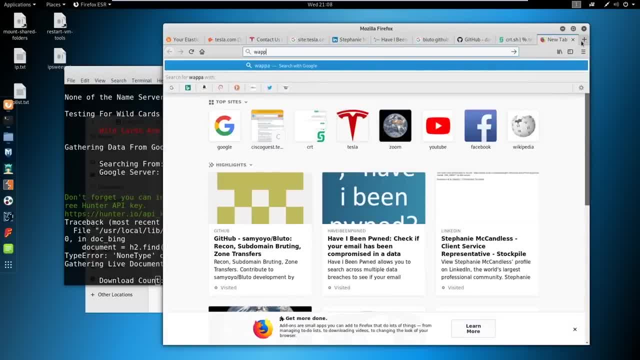 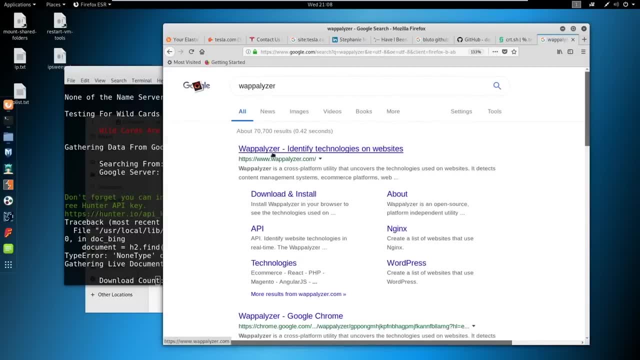 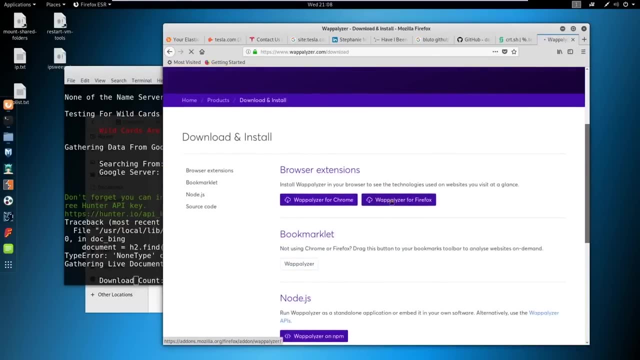 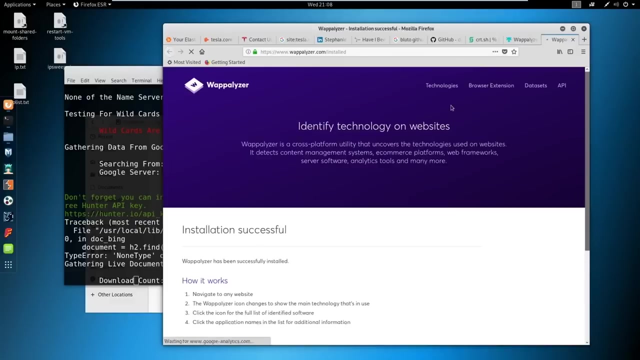 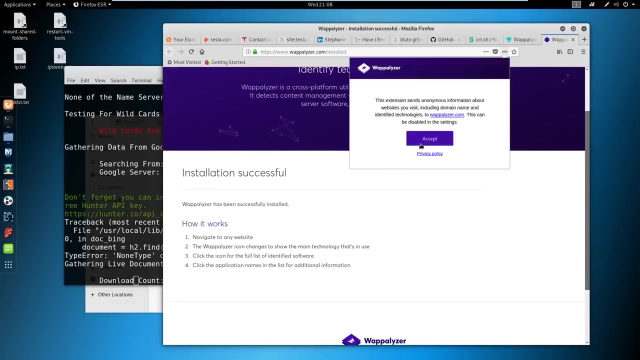 look at wappalizer and if we just say download and install, i actually haven't installed it. we have firefox, let's just do that. we'll add it to our firefox here. add, okay, and here you go. this is our wappalizer. so now let's go to teslacom on this. 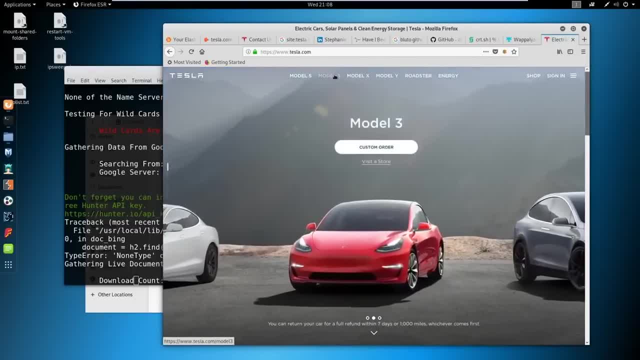 let's see what they're running on. so we've got some sort of javascript framework running tween max. they're using jquery 1.12.4 hgp2. they've got amazon web services- looks like they're running an apache web server. they're doing amazon load balancing and they've got google tag manager. 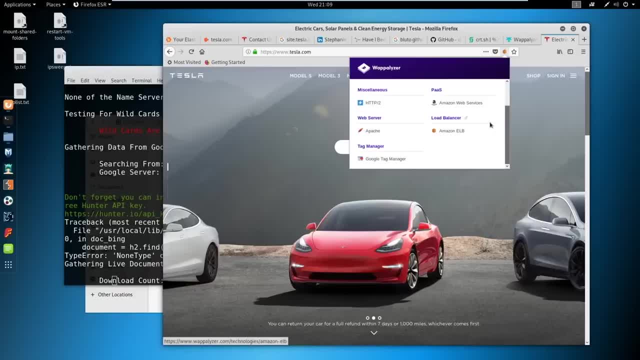 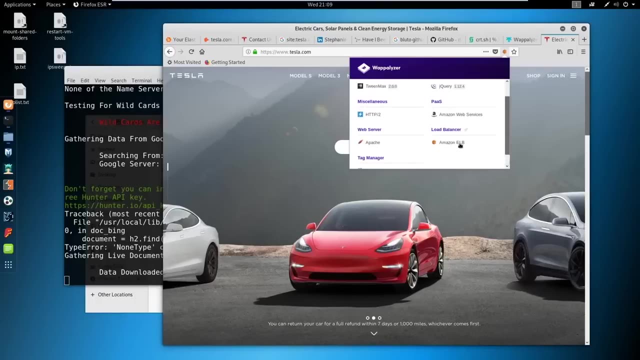 i don't know how heist is running so much. anyways, i did put a rate limit on it, but apparently that's not the case, so maybe i'll have to rate limit a little bit more. but this is some interesting things to look at. here we can kind of get an idea of what's running. 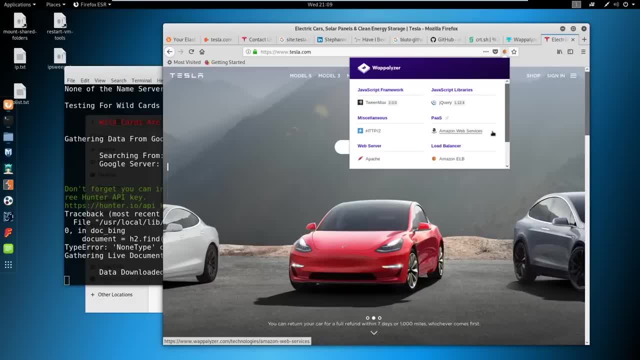 on the front end what's running on the back end. now they could, in theory, put false information in the headers or whatever and try to throw us for a loop right, but we could see like jquery 1.12.4. well, i might want to look up jquery 1.12.4 and see if there's any vulnerabilities with this. 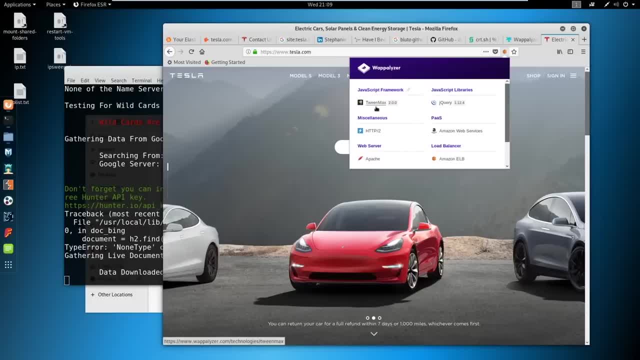 there's been vulnerabilities with jquery in the past. same thing with this tween max 2.0.0. might want to look those up now. it really depends on what you're doing, since this is a network focused course and not a web app focused course. a lot of the time we're worried about the 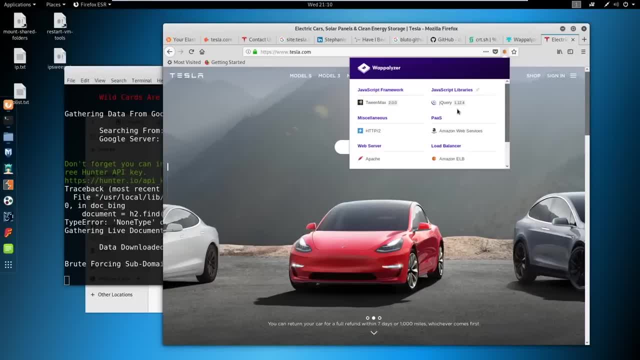 host itself, like i, for example, if we're doing a host and it's on an external and they give us um say, they give us 10 machines, one of the machines happens to be a web server for their website, i'm not going to go on the website looking for web vulnerabilities. i'm not going to be looking for. 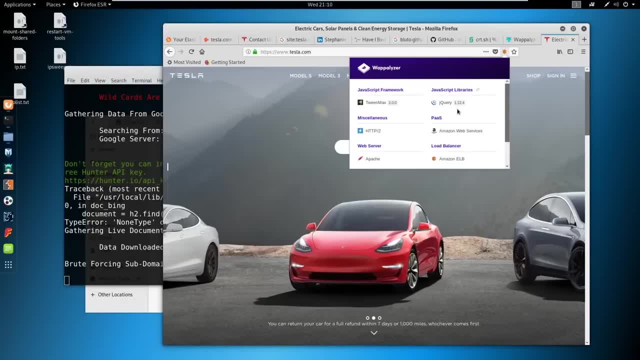 like reflected cross-site scripting. right now i may test sql injection on a login to see if i can get into their system, if it's just a login page, if i can do any sort of bypassing, if there's remote code execution. my goal as a network penetration tester, when i'm given a host like that, is to find: 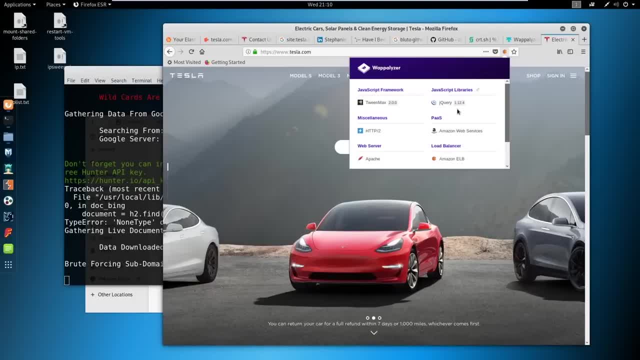 a way in through some sort of code execution. if i find some really critical vulnerability with the web page, maybe, but i'm not looking for it. but if i have a login or some way to give in technically or typically, you're not given credentials for these unless you're doing an external pen test. 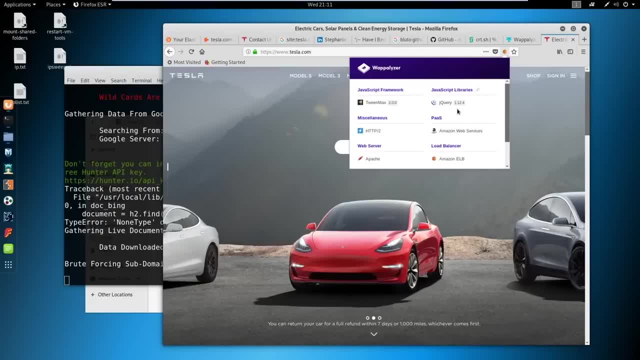 and a web app. now, on web apps, a lot of times you'll get the website and you'll get to do the host that's hosting that website, and that's a little bit different because you're doing like a one um, but do keep in mind that if you're tasked to do a network pen test, keep in the scope that. 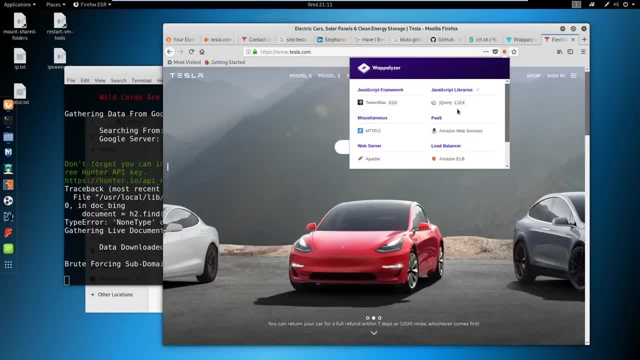 you don't want to waste all your time trying to pen test a website when that's not really the scope of things. so that is the end of my spiel, sorry, okay, so information here. um, we can use other tools as well. let me pull up my syntax, because i don't remember all this, guys. uh, okay, so we can use what. 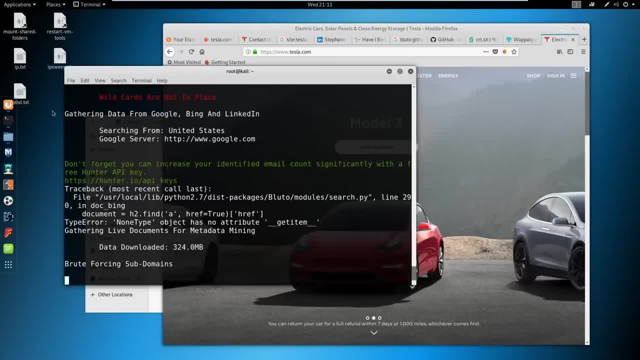 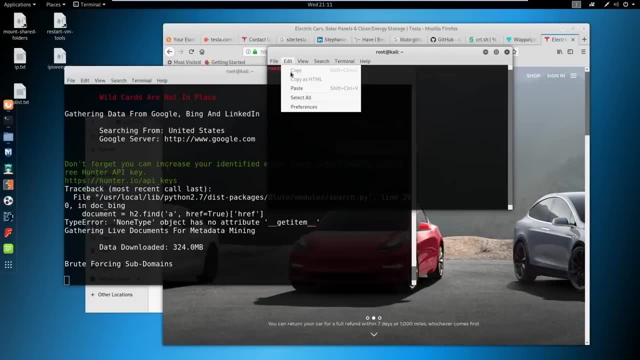 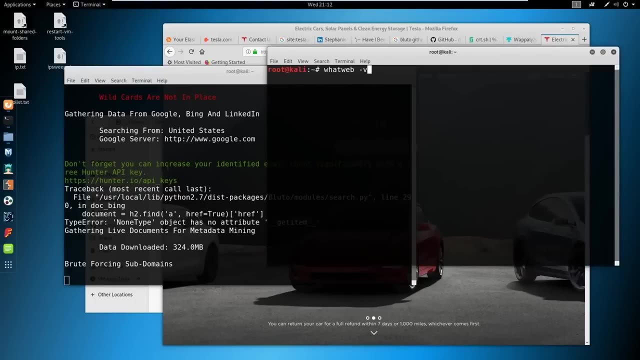 web. so let's check out what web. we'll just say dash v and we'll say teslacom, like that, and it should run against it. now this borderlines to me as active scanning. um, this isn't necessarily passive recon anymore, so we're kind of diving into the deep end a little bit, where we shouldn't be. 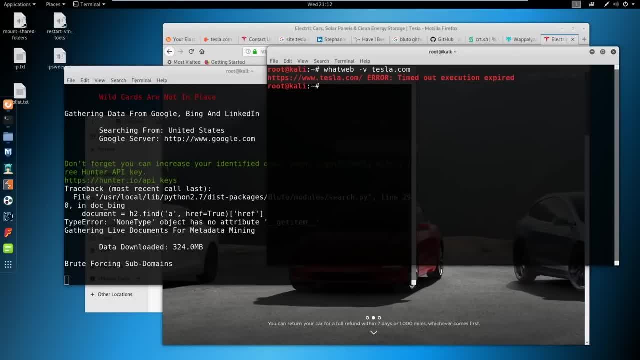 uh timeout execution expired. well, maybe we're not going to use what web. i'm not sure what's going on there way back in old bounty reports. is 100 true as well? thank you, davey, i will note that. um, so you could go to the way back machine see what uh they've had on there in the past. 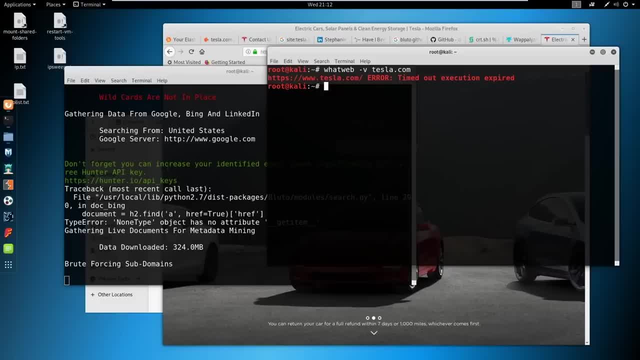 and you also could look at old bug bounty reports. if you look through hacker one or whatever and look for what kind of vulnerabilities they had before, there's a chance that maybe that's still lurking around in other places and you also get a decent idea of what their infrastructure was. 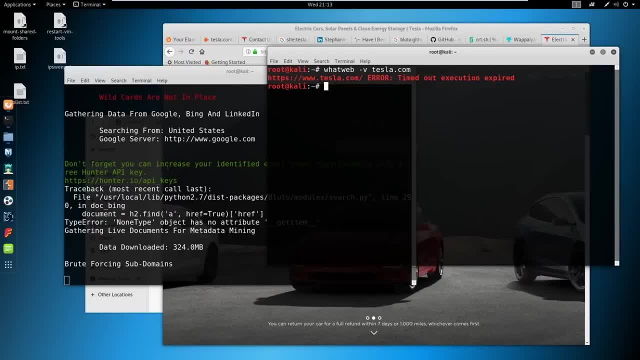 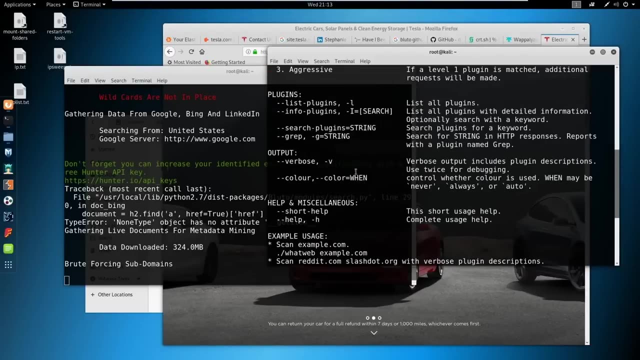 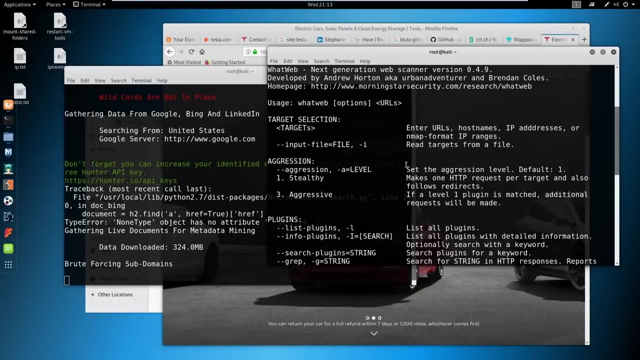 in the past. okay, what web worked for somebody else, so that's good. it said ip. why does it hate me? look at the help. so we did a verbose enter urls, host names, ip addresses or nmap format, ip ranges. uh, all right, maybe i give it an https. 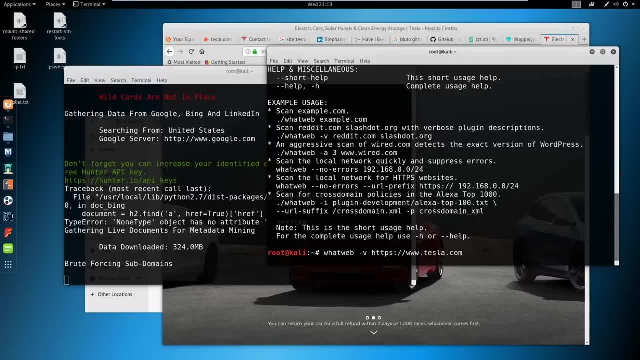 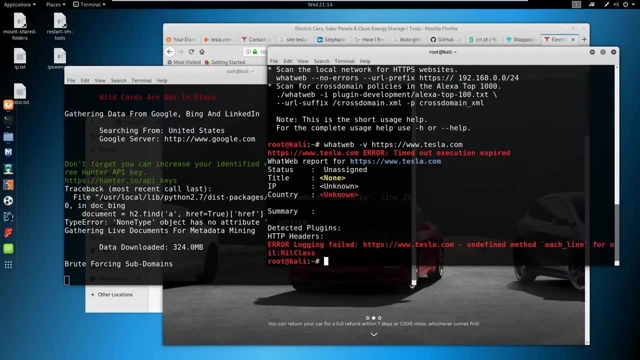 other than that i'm i'm at a loss. i'm not gonna try to troubleshoot what my issue is. ah, i got nothing, guys. it hates me, everything about me. well, at least it's working for you. okay. other people are saying my syntax worked for them, so good for you, guys. 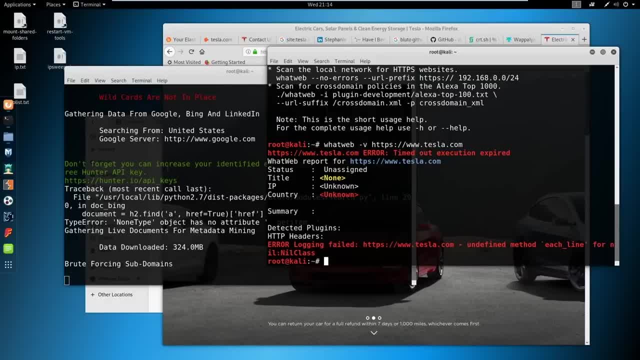 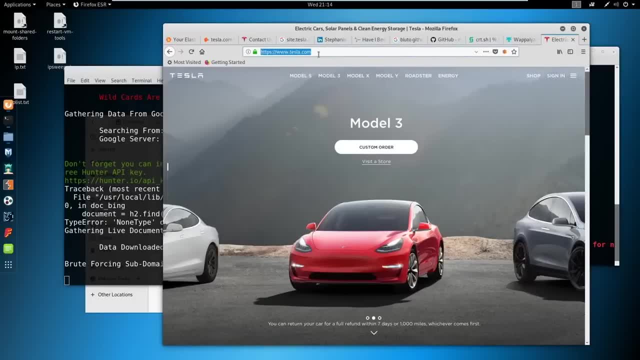 uh. so other tools we can use. we can use. builtwith is another tool and that's a website. now there shout out to tim tomes. i did attend one of his web app classes last year and he really turned me on to the idea of being able to really fingerprint. 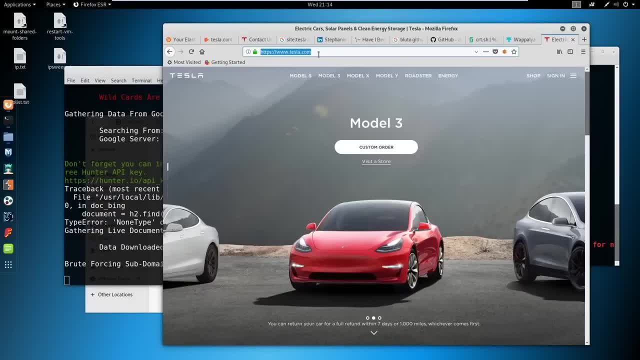 and almost scan without scanning a website, site or you know, like a domain. So there are, there are sites out there that will tell you information without you ever being associated with scanning that site. This even goes out to open ports and things like that. So it's really kind of cool that you don't have to associate. 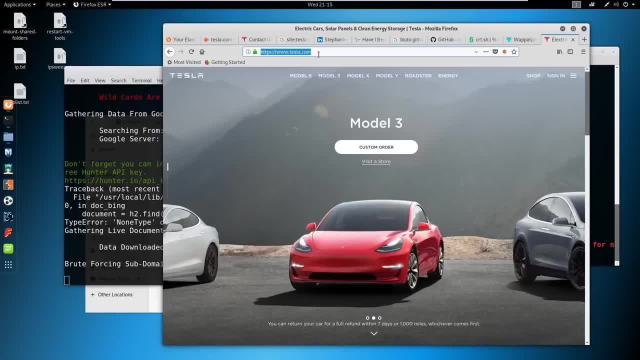 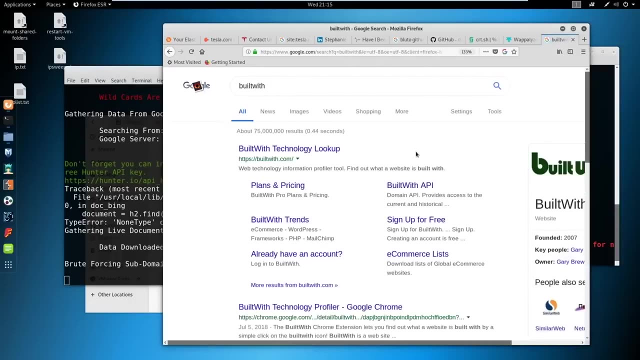 your IP if you don't want to, if you want to do data digging other ways as well. So let's take a look at built with. Yeah, they're going to see a lot of increased traffic And they're going to be like what the hell is going on? Somebody's going to point them to the. 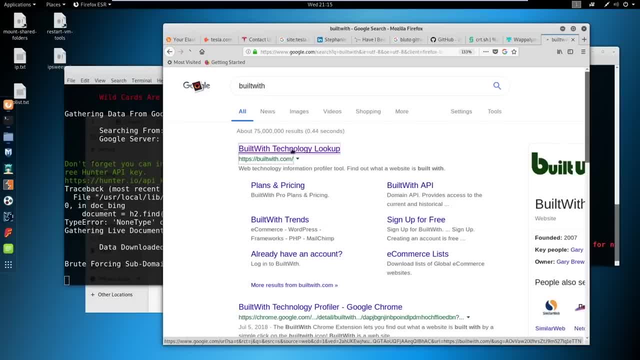 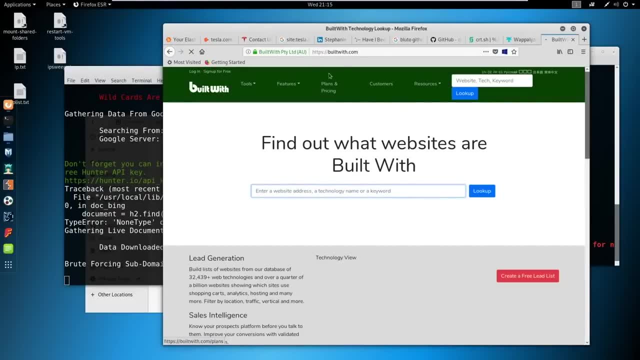 stream and then I'm going to get sued And there's not going to be any more of our of our hacker streams. guys, All right, built with dot com And we'll just search Tesla dot com. Can I get sued for this? I don't think so. I'm just being dramatic. 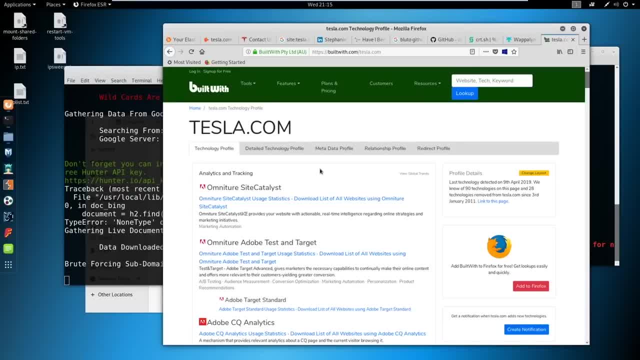 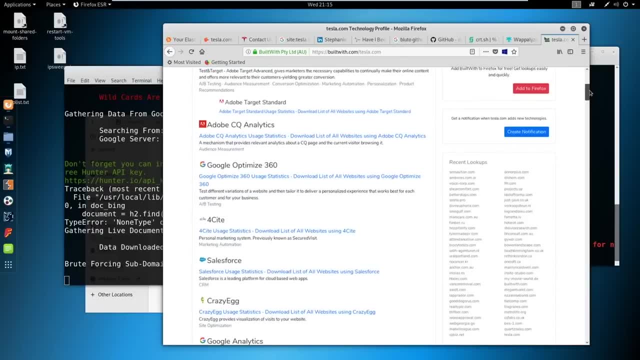 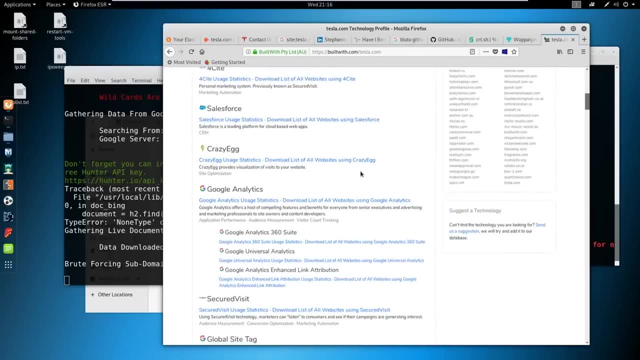 Cookies in jail would be good, though. OK, so there's a whole lot of junk in here that we have to sift through, But it kind of tells us some of the things that might be interesting. They're using Salesforce, something called Crazy Egg, Google Analytics. 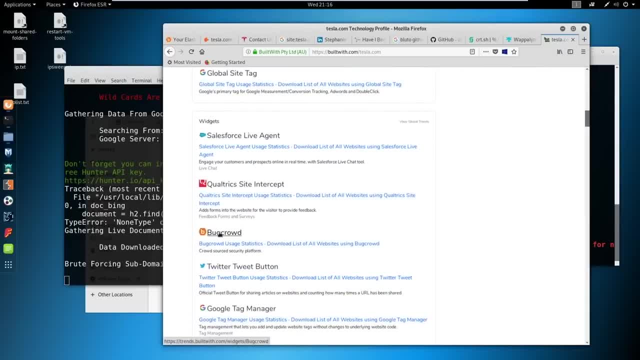 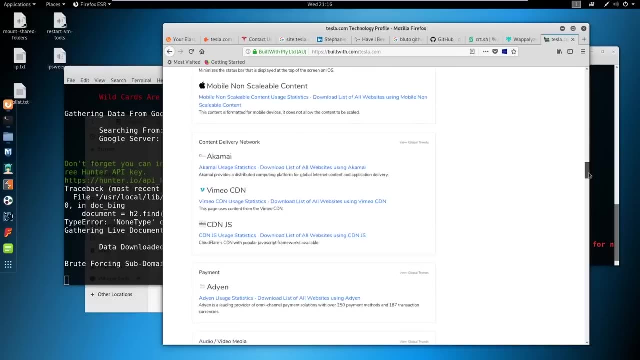 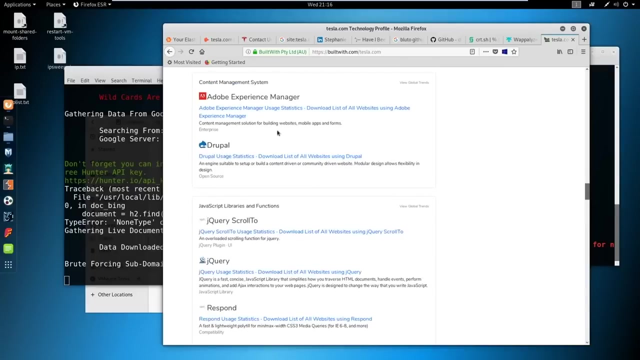 they've got widgets: Salesforce widget, Obviously. they're on Bug Crowd that shows up here. They're on Twitter Qualtrics, Some mobile information, content delivery, payment information. They've got a content management system of Adobe and Drupal. I mean, there's a lot of. 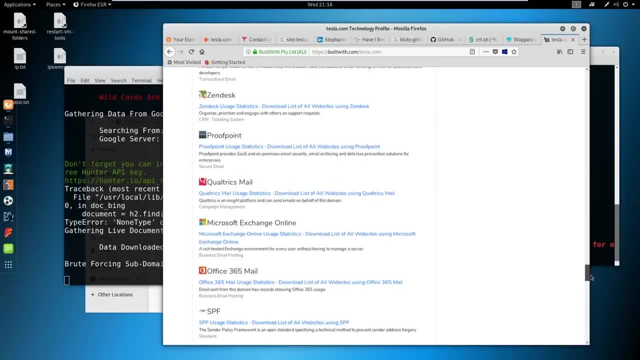 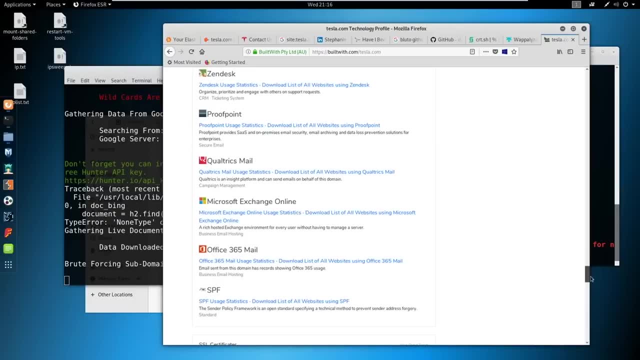 information here that you can dig up, And we never had to go onto their site. They've got a ton of different email hosting providers, which is interesting, So it looks like they got proof point for email security. So I mean, this is all all very, very useful Shows who their SSLs are through. 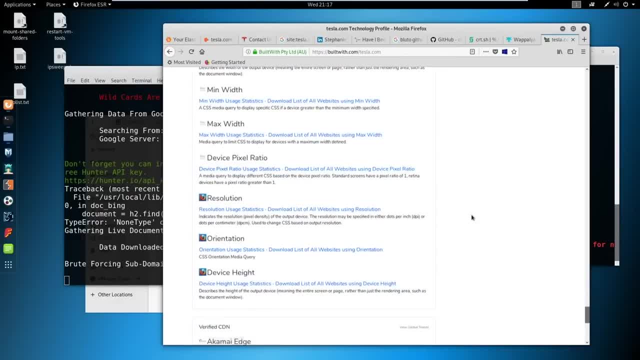 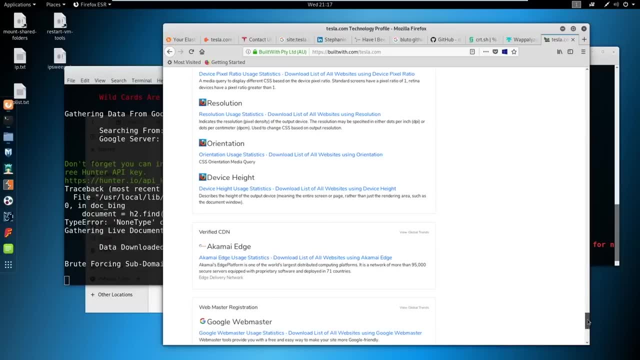 their name servers are through. So I mean you could go through this and try to pick up a way to really map them out and what they're using. Yeah, email security. I've gotten past proof point enough times in my life. 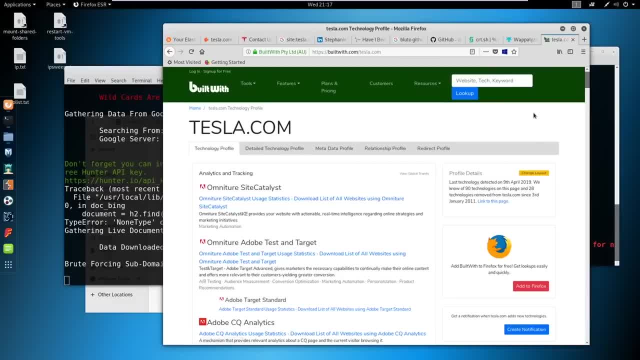 OK, so we are at a point now where we have gathered quite a bit of information. Is there information that you guys have gathered for me? Has anybody gathered? I'm just curious. more than anything, The WhatWeb scan scanned a totally different website for you. Well, that's not reliable. 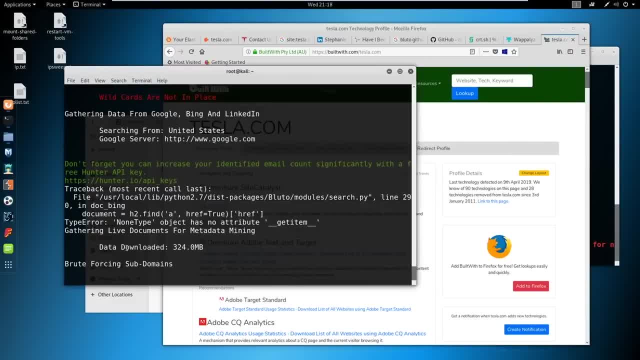 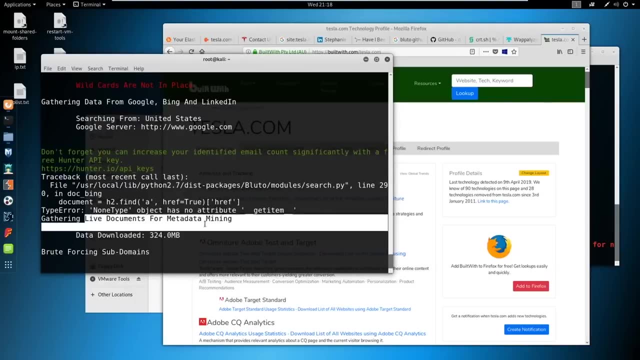 You found the CEO's name. Oh man, It appears they built some kind of car. You guys are a bunch of jokers. Let's see where we're at. So gathered some metadata for mining Data downloaded: 324 megabytes. It's quite a bit of data. 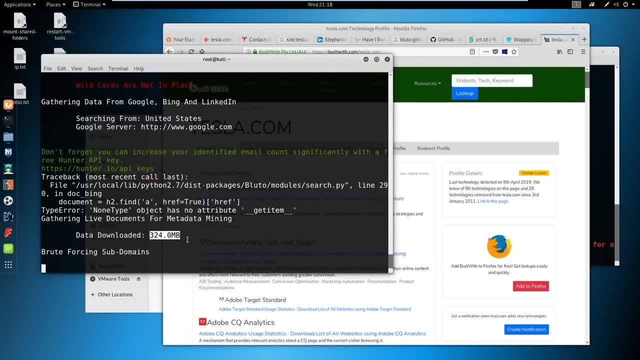 Is anybody past this point in their Bluto? Has anybody's Bluto got past the brute forcing of subdomains? What exactly are we brute forcing? So what it's doing is it's taking a list And it's brute forcing the subdomain So it might have just a common word: list. 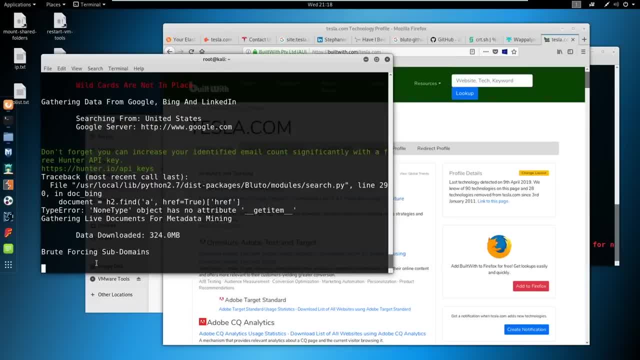 like, say like careersteslacom, So it's going to go through the list and see what resolves and what doesn't. You guys want to social engineer me. You guys are on my Instagram earlier Got kicked off by the VPN. Is that bad? I don't know if this has anything to do with your. 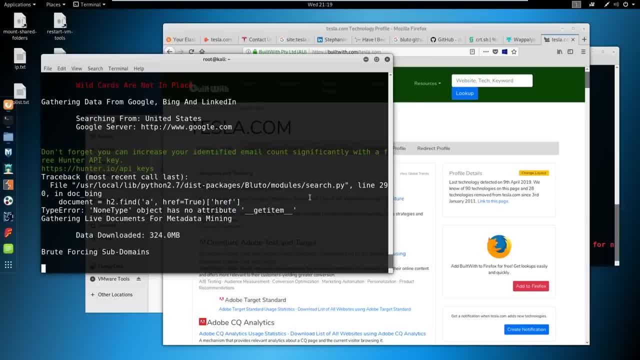 your VPN kicking you off? Yeah, definitely. download the password list. You're more than welcome to use my script. improve my script. Give some credit where credit's due. Don't just steal the script, even though it's terrible. It's not hitting a login field, Jake, So what's happening is it's searching the subdomains. 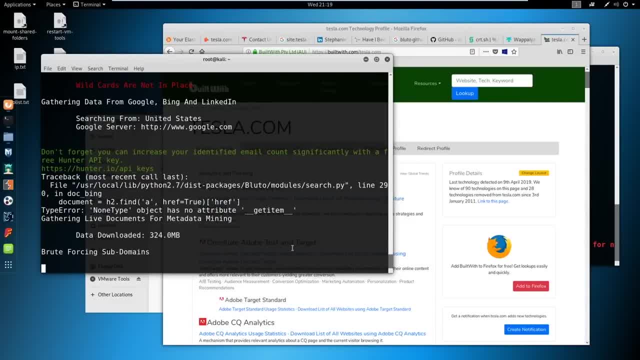 and it's looking for a response code, right? So there's different HTTP response codes. So if it 404s, then it's no good, right? But if it gives us a 200, then it's likely good. If it gives us a 302, a redirect, then maybe it's good, Maybe. 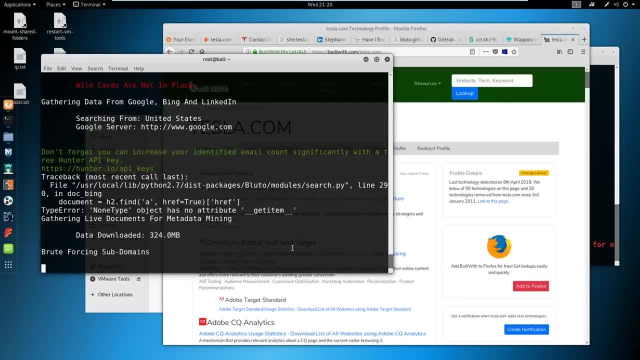 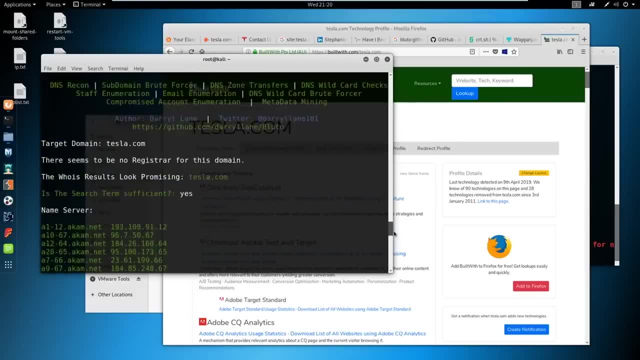 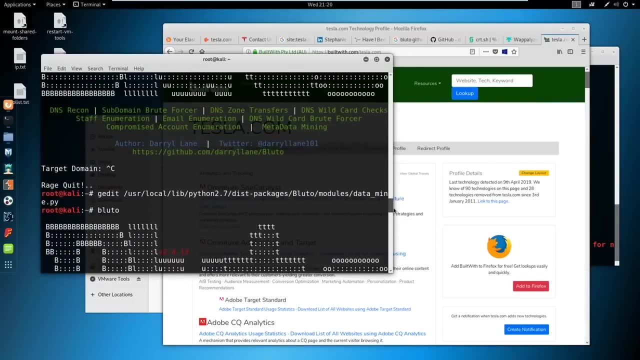 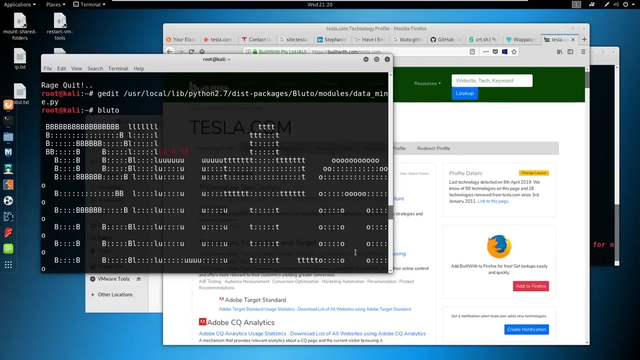 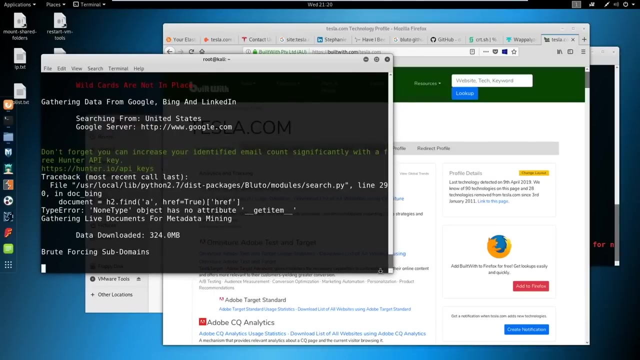 it's bad. We'd have to check into it. What was the line we needed to correct on Bluto? It is for the OLE. There should be something about OLE OLE file. Did you catch that Good? All right, I think I've shown you guys pretty much enough for you to get the idea of what we're. 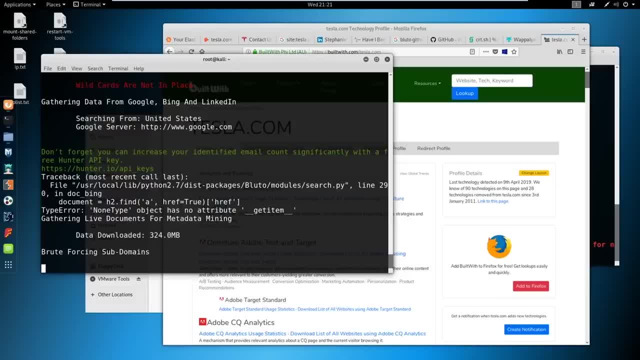 doing, Like I said during the little PowerPoint, we're not going to cover all the tools or problems. We're going to cover everything. We're going to cover everything. We're going to cover probably even a quarter of the tools, But what we're doing is identifying some of the processes. 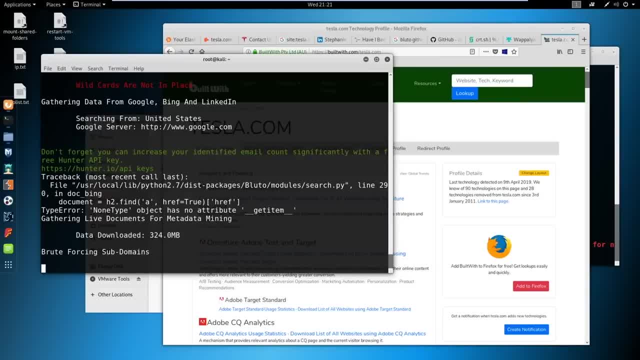 that we would do And really the takeaway is that information gathering is important, Finding the breach password list, like we did, that's going to become really important on assessments. So when we get into that in our later episodes, you'll see how we can actually. 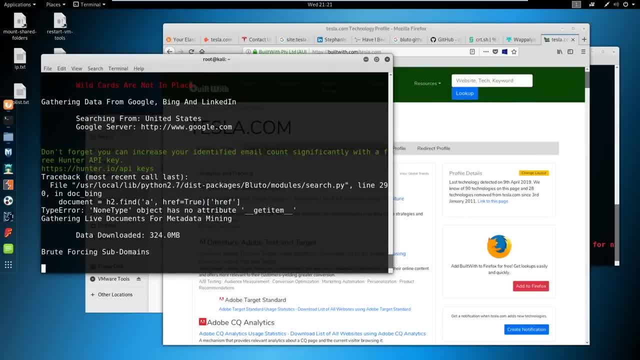 exploit that, But just keep thinking about these things. Think about information gathering. If you're ever asked to do physical assessment, think about looking at Google Maps satellites doing some sort of recon, going through pictures. Twitter and Facebook are insanely good for just finding these pictures of badges or desks or 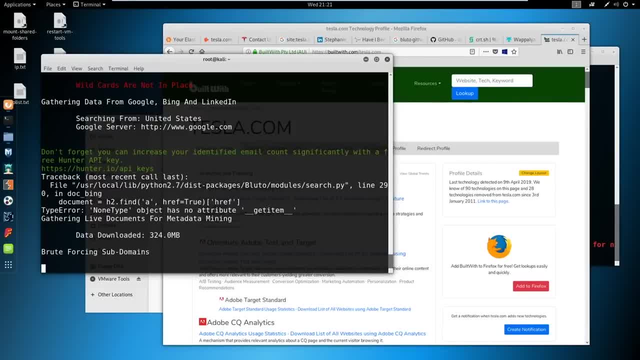 anything that you can. If you're doing red team assessments, you get a lot more time to do those sorts of things, But when you're doing a limited penetration test with the time limit and everything else, it's hard to do the true information gathering. So if you're ever asked to do physical assessment, 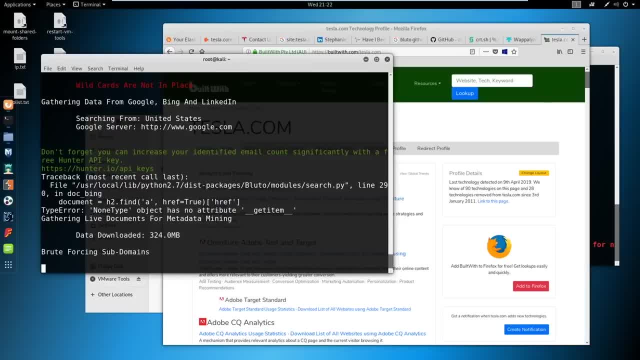 it's hard to do the true information gathering, depending on how big a company is that you would want to do, But these are some things to think about: trying to find as much information as possible, doing target validation, fingerprinting, finding subdomains, breach data, etc. 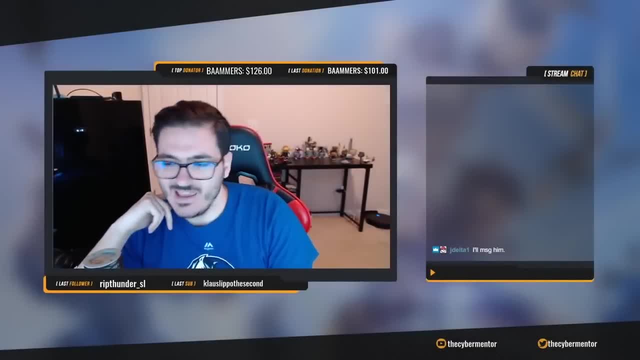 Tonight's agenda. we are going to be talking about scanning mostly, So we're going to be doing some scanning In order to talk about scanning. we're going to be talking about scanning mostly, So we're going to be doing some scanning in order to talk about scanning. 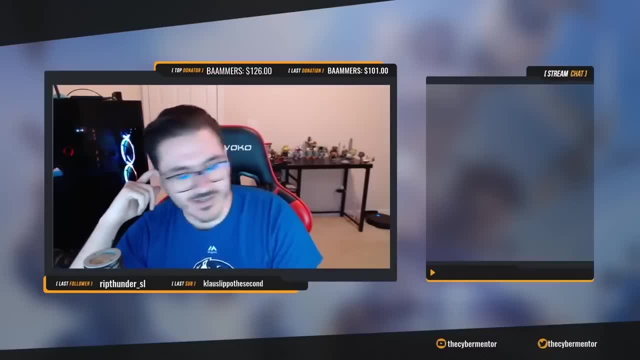 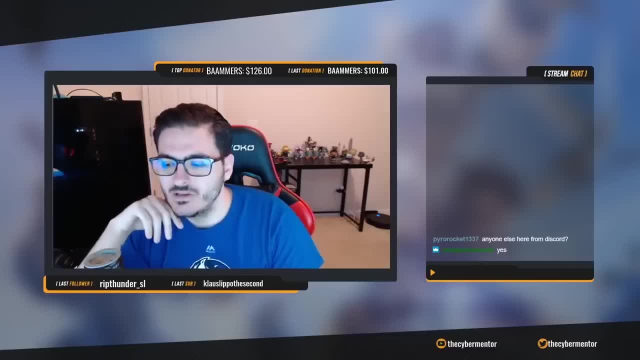 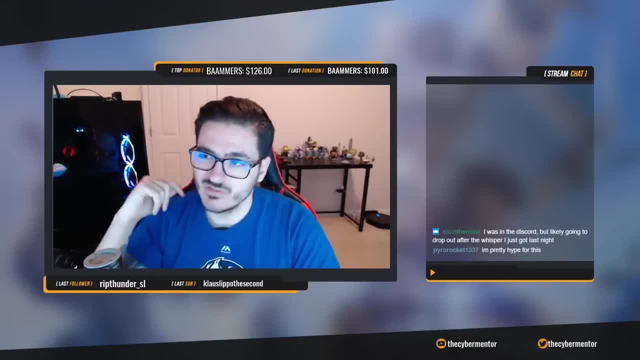 to cover Nmap. We're going to cover some Metasploit. We're going to get into your first lesson or introduction to Metasploit, which is a tool we haven't seen yet but we will use a lot, So we'll cover quite a bit. 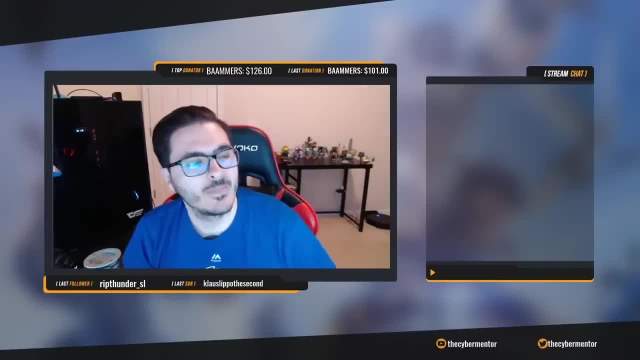 Okay, let's talk TCP versus UDP real quick. So when we do port scanning, typically we're going to be scanning on the TCP side. However, it would be incorrect of you to not scan the UDP side as well. There are some tools that only run on UDP, some protocols that only run on UDP. that would be. 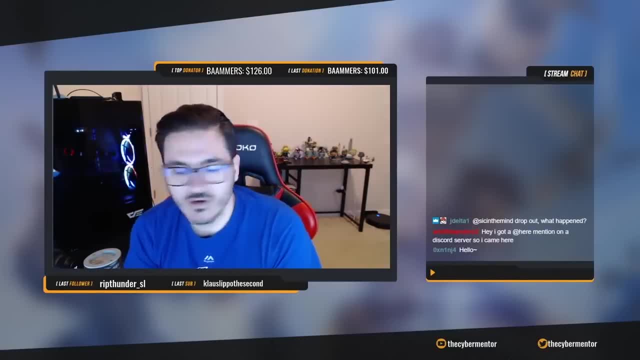 important that you would not want to miss if you're doing some scanning. So when we talk about TCP, TCP is connection oriented. It has a handshake right. So we're talking about that three-way, Three-way handshake. So we're going to talk about that, We're going to see a live view, We're going. 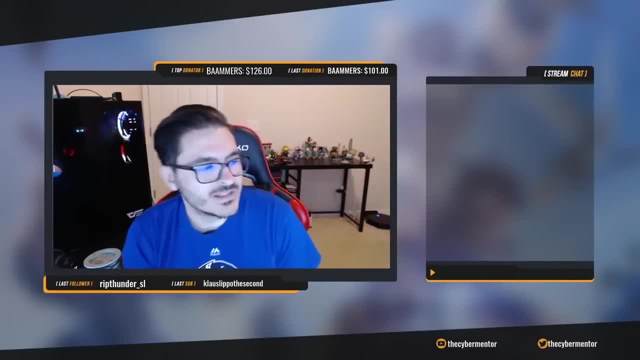 to use Wireshark tonight and see what that looks like, And it's used on applications requiring high reliability. So some examples of that would be HTTP, FTP, Telnet, anything that you would need some sort of connection to right. On the other hand, you have UDP, which is connectionless. 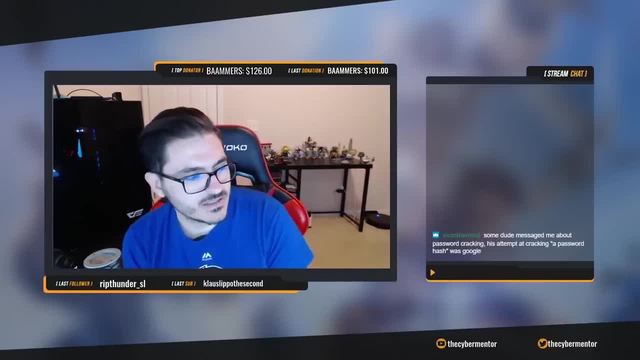 It doesn't have a handshake And basically it's used on applications that require a fast connection. So DNS, DHCP, SNMP- really we don't need high reliability for these protocols, right? We just need some sort of fast connection. So with that much said, we're going to cover TCP. 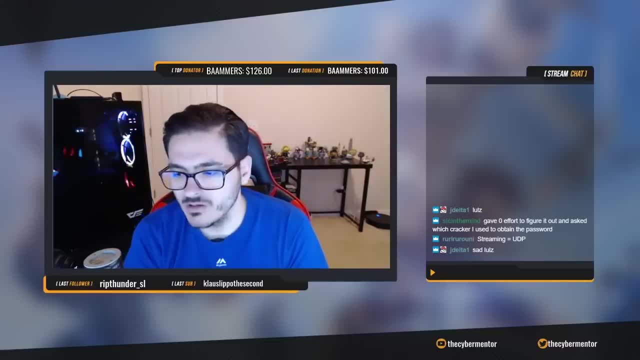 and UDP more in depth as we go along. Let's just get right into it. So let's kill this. I've got my Kali session up here. We're going to go Full screen. Ah, the jokes. I love the jokes. 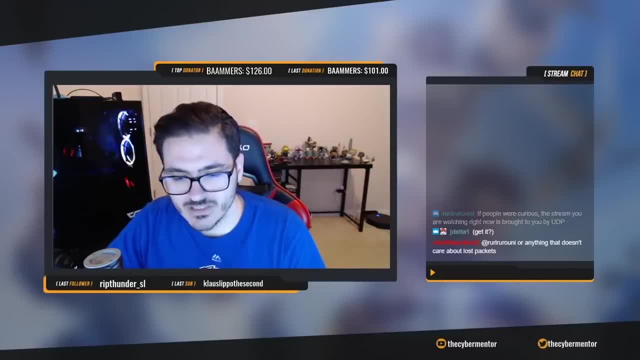 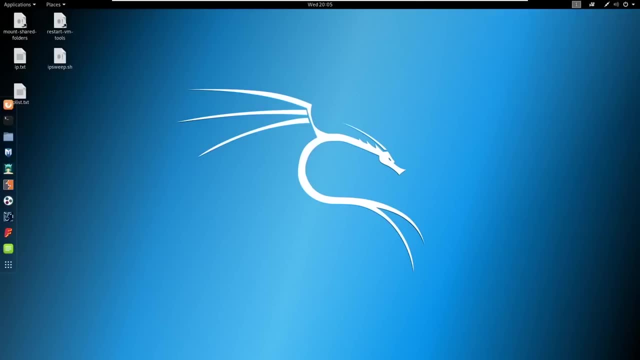 And I realized that I just did that whole PowerPoint presentation and didn't switch the screen because I'm a terrible person, Terrible. I'm off my game tonight. You don't need the PowerPoint. I'll throw it up for a quick, quick second though. 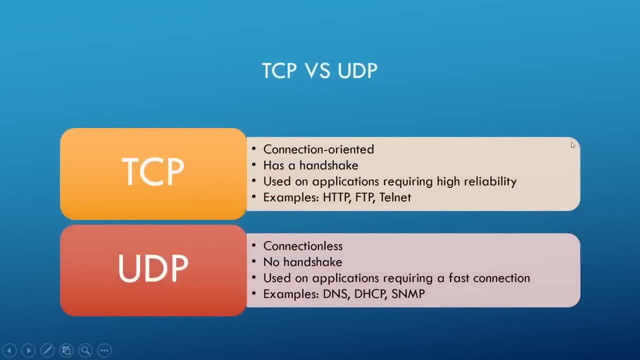 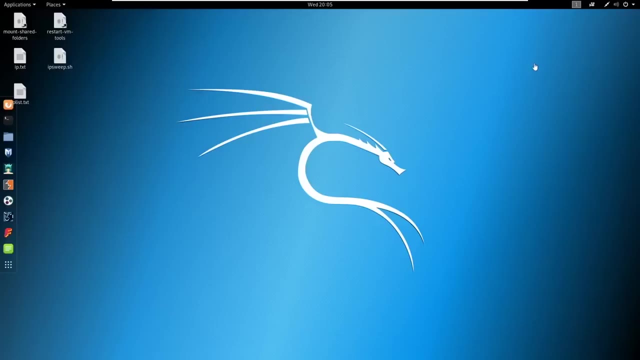 just so you guys can see. There's the cute little chart I made for you guys. Yeah, I'm a pro streamer, So here's your little chart. If you need to see that, you could pause the video later on. Cheers, Okay. So now going into our lesson. First, we're going to talk about the three-way handshake. 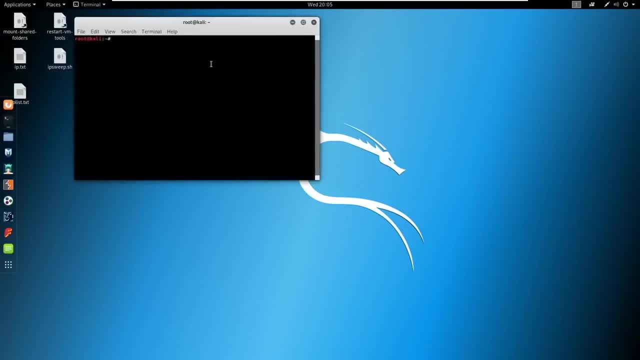 And to do that, we're going to open up Wireshark. So let's do Wireshark And let's type in an ampersand after that, And we're doing this just so we can start up a process and run it. 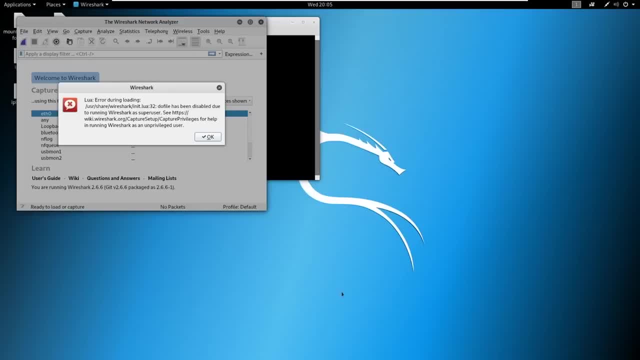 And if you get an error, that's completely fine. No, that link isn't valid. I realized that I need to change that link. Sorry guys, Here I'll shoot you a Discord link right now. I've made some minor changes. Actually, if you go to the website, you can. 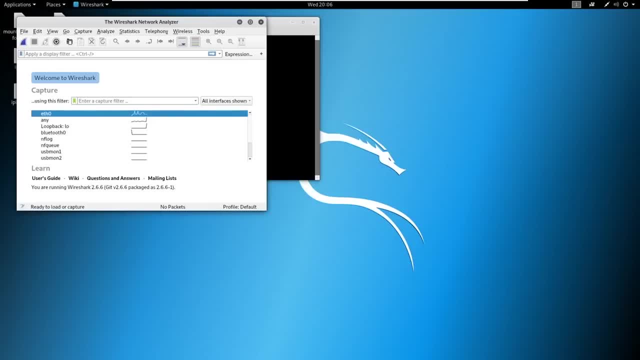 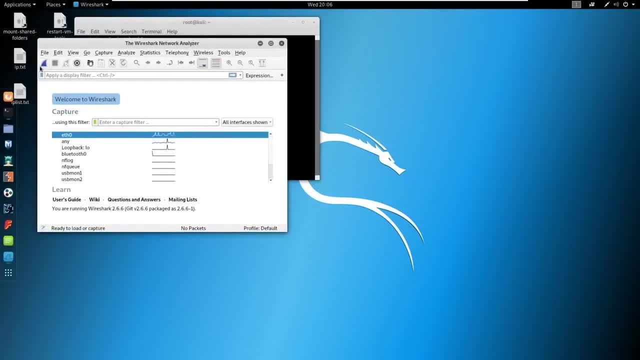 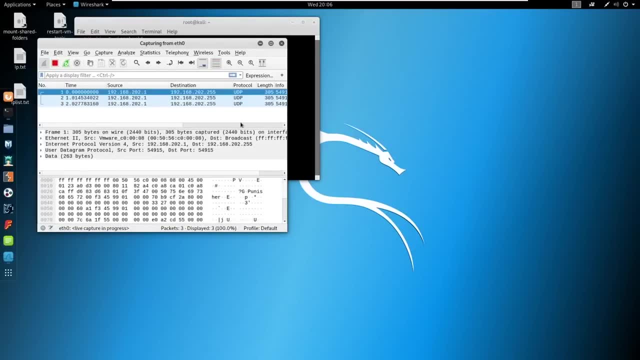 Okay, So we're in Wireshark. All we're going to do here is just hit, start capturing. Make sure you're on your ETH0.. You're going to see a bunch of stuff starting to come through, But this is UDP protocol. 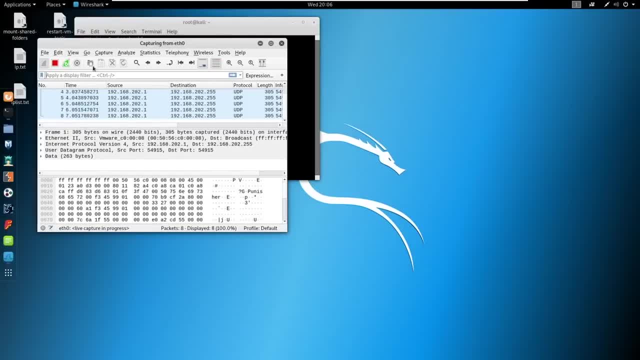 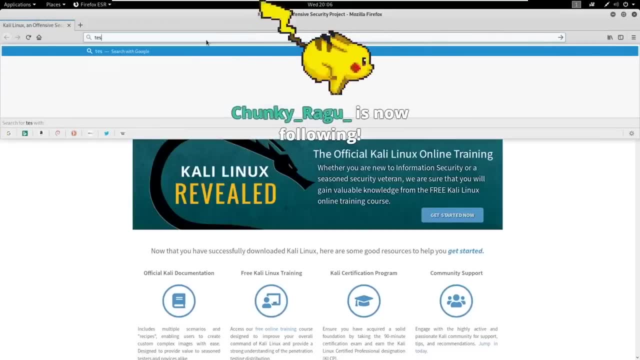 We need to make some sort of connection. So what we're going to do is we're just going to go out to the interwebs And we're going to just go to a website- Our favorite probably- teslacom right from last week. 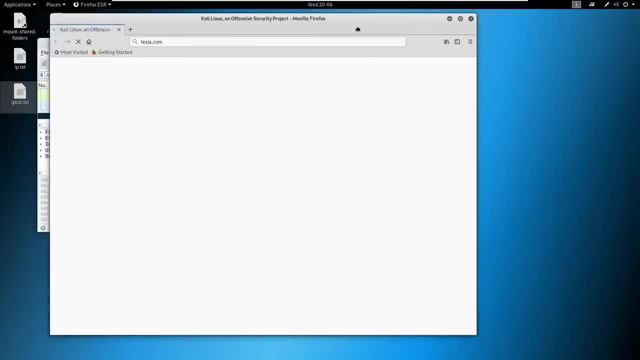 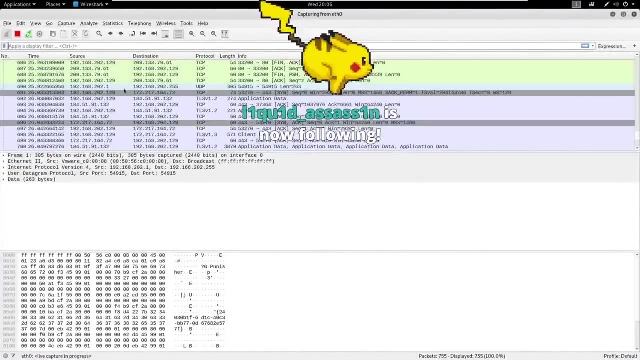 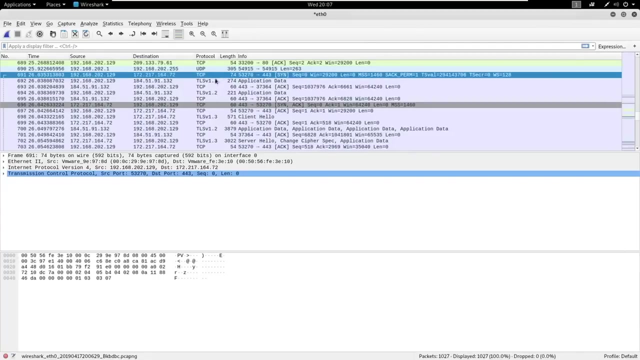 We'll make that connection. Okay, And it came through in here. There we go, Okay. So my guess is that 172.217.164.72 is the Tesla website, just on a hunch. So when we're using Wireshark, what we're 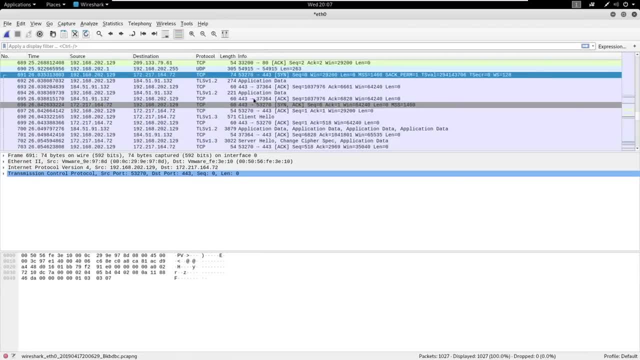 doing right now is intercepting traffic. If you've never seen that, we're just kind of listening in and capturing all the traffic that's coming through. So when we talk about this TCP handshake, we're talking about a process that goes SYN, SYNAC, ACK. So what happens is over TCP. 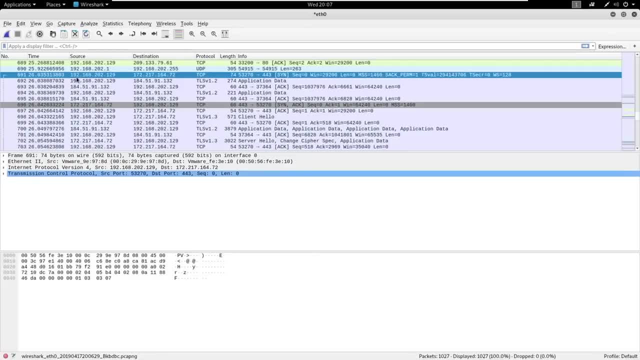 you see right here where we're starting. you see, my IP address of 192.168.202.129 is reaching out to this destination and saying, hey, I want to connect to you. So this is what is considered a SYN packet. 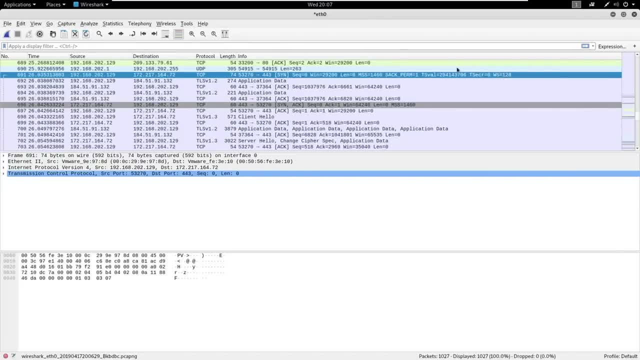 We send a SYN packet out. Now the application reaches back out to us And it says: hey, I see your request And I'm also going to acknowledge it. So here's the ACK And this is where SYNAC comes from. Once we get that acknowledgement, we know hey. 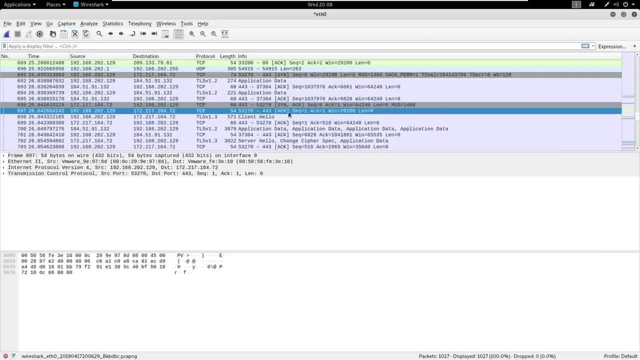 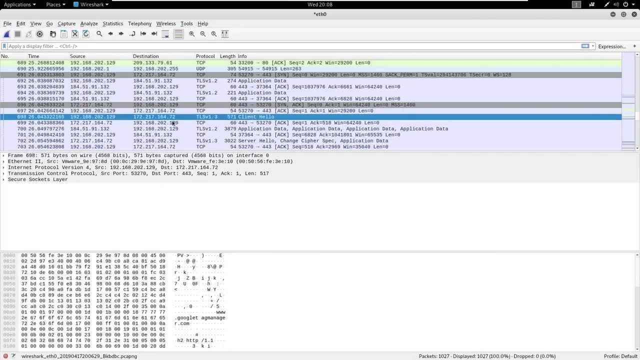 that port is open, We can make that connection. We're going to go ahead and send an ACK back to the client one more time here And we're going to say, OK, The client says hello, meaning we've fully established that connection. So when we do scanning we're going to be using 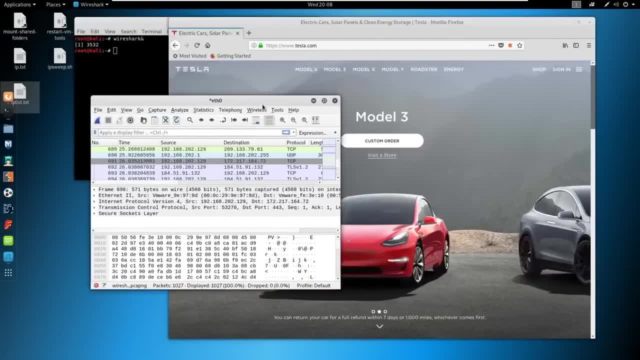 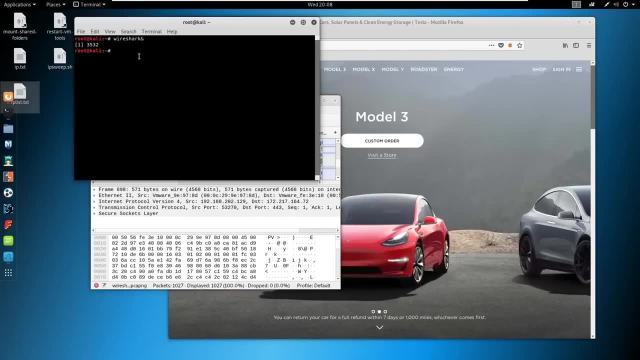 NMAP. Now NMAP works a little differently. By default it's running something called StealthScan, And you might have seen it something like SS right with the StealthScan in the past. We don't have to use that anymore. Somebody here taught me that. 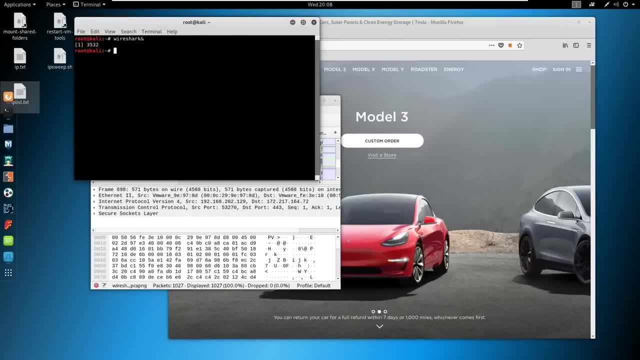 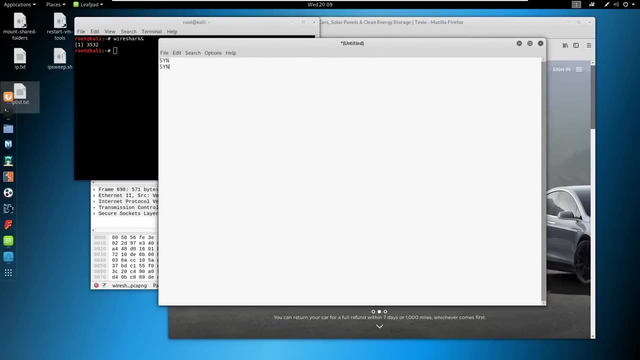 a few streams back. So when we do a scan here let me open up just a little leaf pad. When we did the original right, we did a SYN, we did SYNAC, we did ACK. OK, When we do StealthScanning, we say SYN, the port comes back and says SYNAC. 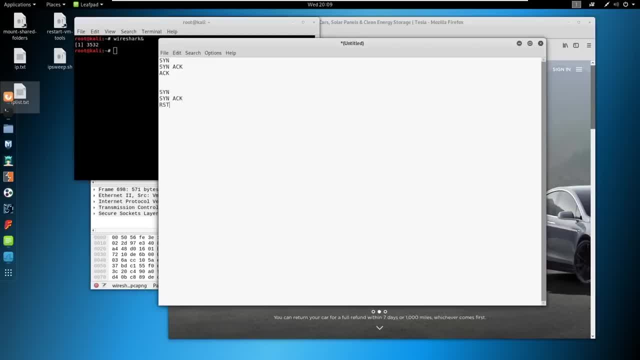 and we send a message out that says RST for reset. Basically, we say: just kidding, Now this is no longer that stealthy. Maybe it was stealthy back in the day, It gets picked up, But this is the most common way of scanning- is sending that reset. So what we're doing is we're 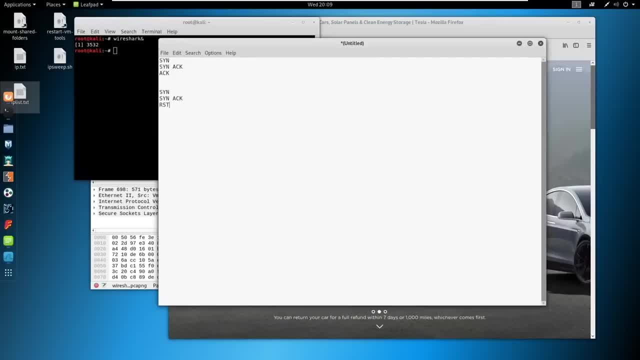 reaching out for connection. The client says, yeah, that port's open, I'll let you connect. And we just say, hey, just kidding, I don't want to connect, But Nmap will come back and it'll say: OK, well, that port's definitely open. So 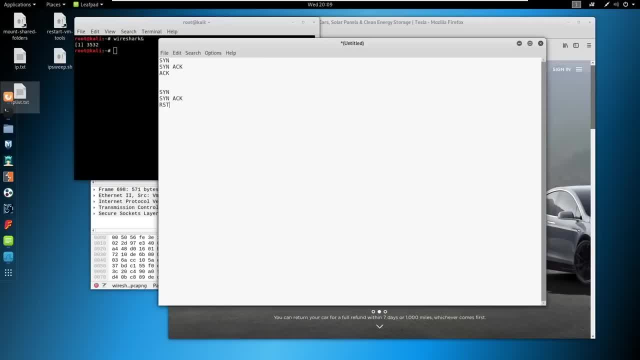 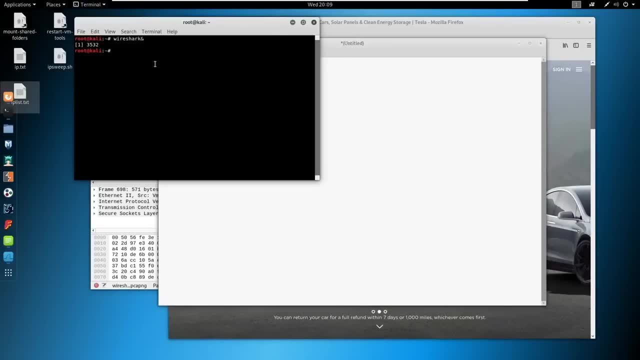 here you go. I'm going to report on that. All right, JDelta, I'll get a hold of you after that. I'll message you somewhere, all right? OK, So let's go ahead and look at our first scanning tool, So the most common scanning tool, you're. 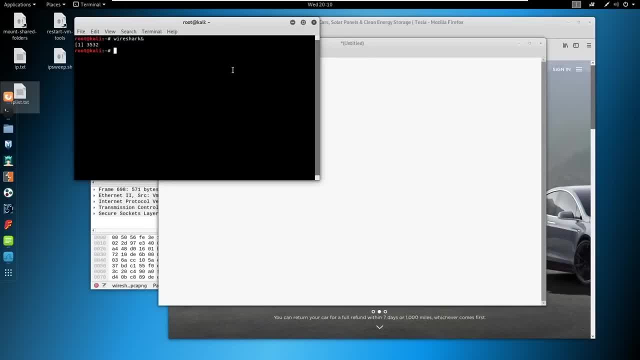 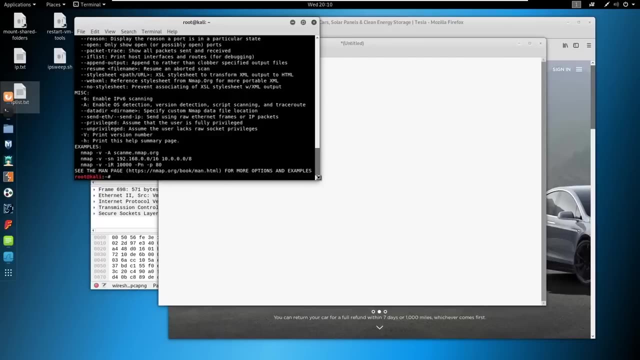 going to be seeing is going to be Nmap, So it stands for Network Mapper, I believe, And we can just type in Nmap like this: do a dash, dash, help, And we can see all the resources. And let me blow this up for you guys here: 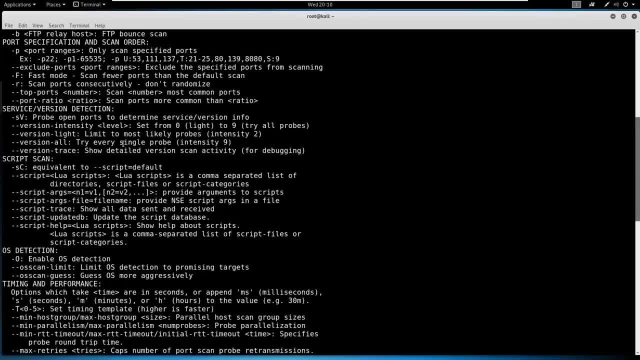 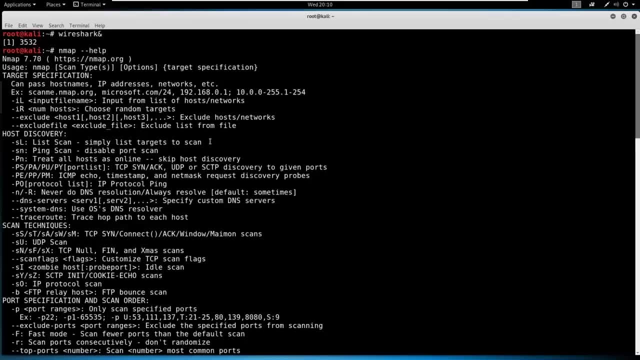 We can see all the resources that Nmap has to offer. So I'm already seeing it come through in the chat. People have their ideas of what they like to run. They run different things. I'm going to show you the Cyber Mentors method. It is not the best method. 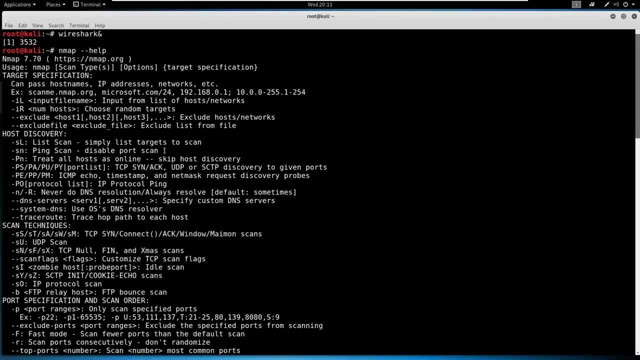 It's not the worst method, It's my method, right, So you might see some videos of me doing it. I'm going to show you the and map method. I'm going to show you the and map method. I'm going to show you the and map method. 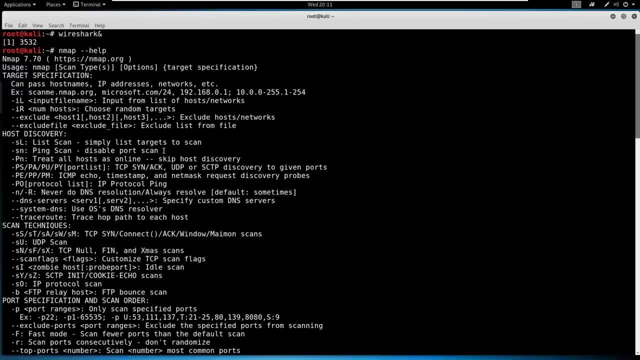 some other ones. come through, check them out, find what works for you. I'm going to give you some tips and tricks and ideas that I like to think about, And you can kind of take my ideas and go wild with it. So when we're looking through here, we've got a few things that we can do. We 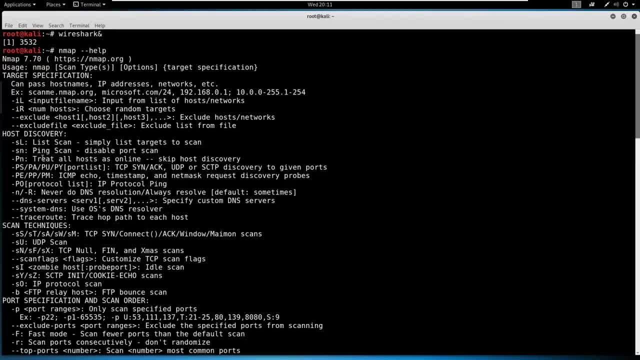 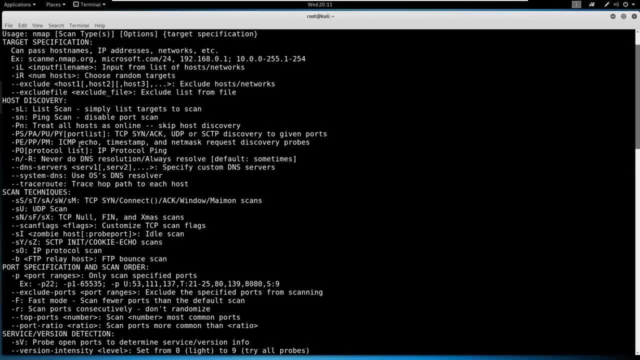 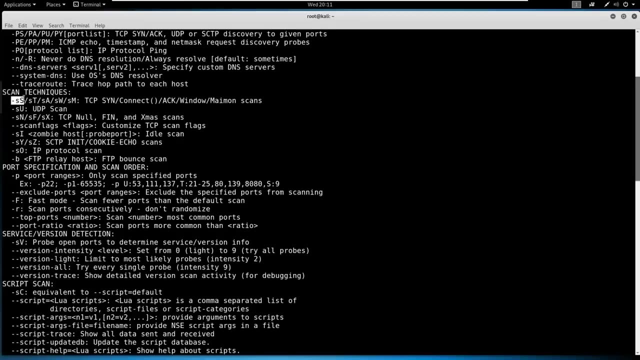 can do a ping scan like a port or a ping sweep. You've got a few things like this capital PN I've used before just to treat all the hosts online. Really, we're curious about scanning techniques. The most common, like I talked about, is the stealth scan in here, But they've got quite a. 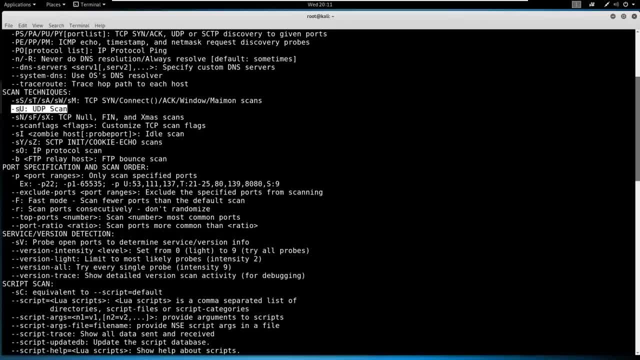 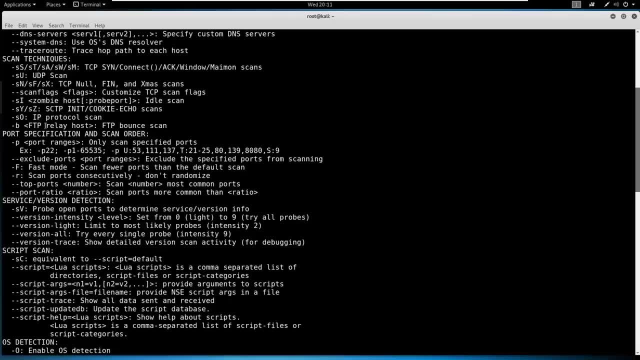 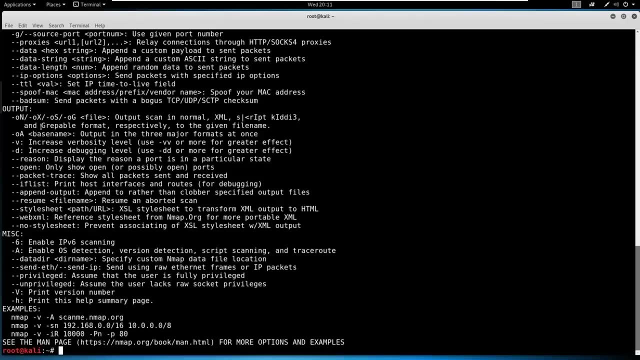 bit that you can search from. Same thing. the UDP scan has its own flag. They've got some special ones, like the Christmas scan that's in here. So really we're going to focus on just my syntax, But if you need help with syntax, you can come through here and look at some of this stuff. One. 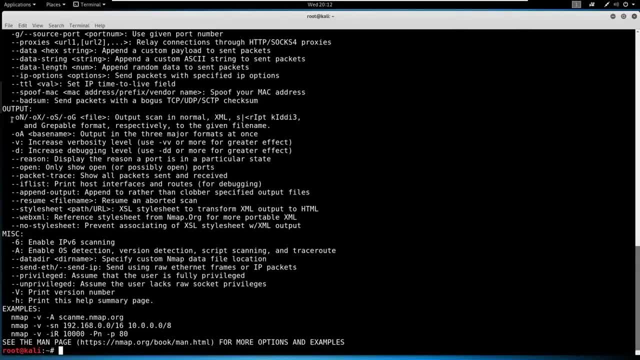 of the most common things I've used before just to treat all the hosts online. really, we're curious about scanning techniques. The most common, like I talked about, is the stealth scan in here. more important ones too, is this output: if you want to save your stuff to a file, a dash on, we'll put. 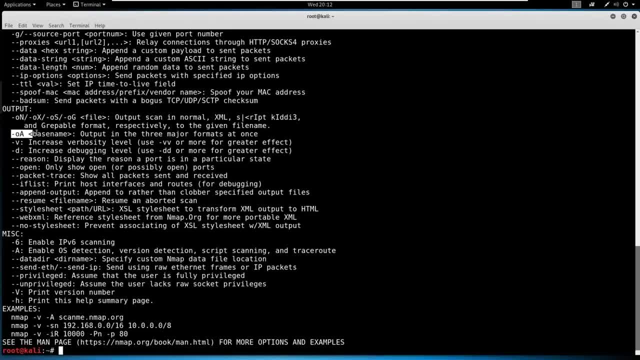 it out to a normal file or a text file. you could do a dash oa to put everything out to all the formats, and we'll talk about that in just a little bit. somebody asked: is there going to be a q a session after the course? yes, there will be a q a session, all right. so what i'm going to be doing? 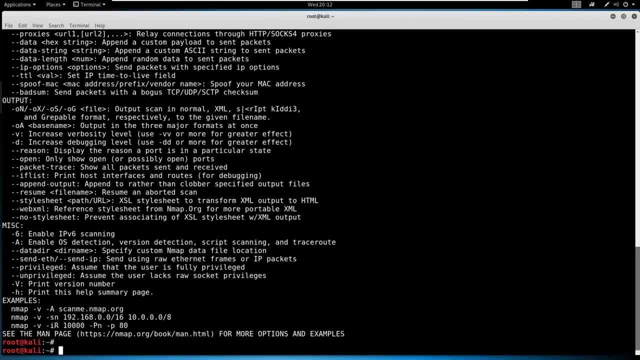 is, i'm going to be scanning an ip in my network and then later on we're going to be attacking tesla again, staying in scope, of course. so first and foremost, we need to find what ip addresses might be up in our network. so we're going to do what is called a ping sweep, if you remember from. 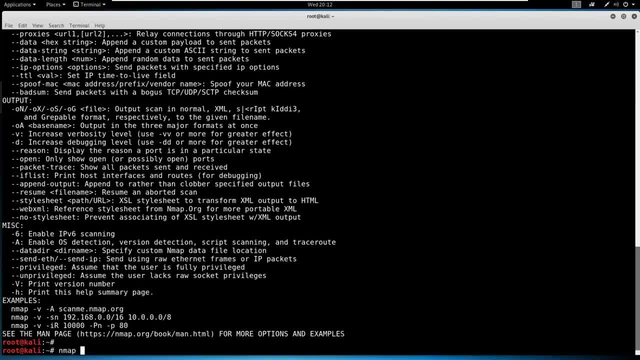 the first video, we built out our own ping sweeper and you'll notice that when we use nmaps- ping sweep- sometimes it's not all that reliable, so i'm going to just sweep my whole network, something like this. so all i'm saying is nmap. i like to think of sn as sweep. 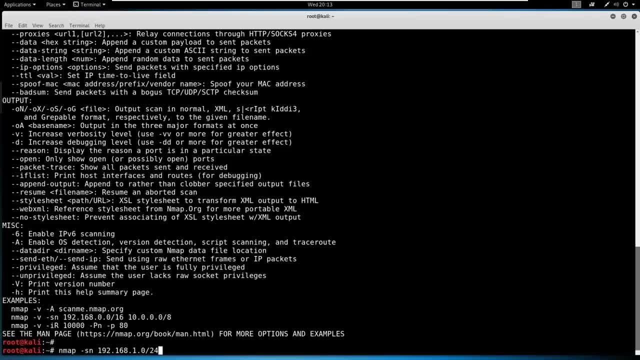 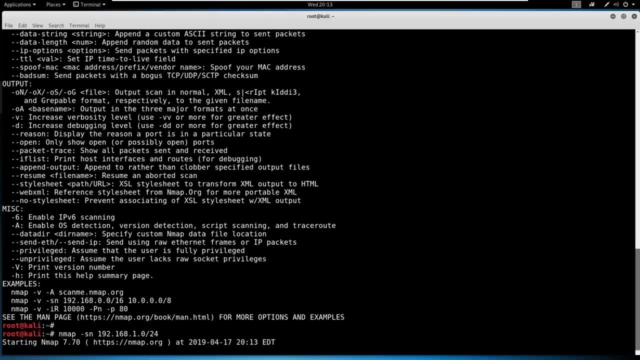 network- i don't know what it stands for- and then i put in an ip address here and all we're going to be doing is sending out those icmp packets and saying, hey, are you up? and we're going to go ahead and send that out. it should be relatively quick. some of these we're going to let just just scan. 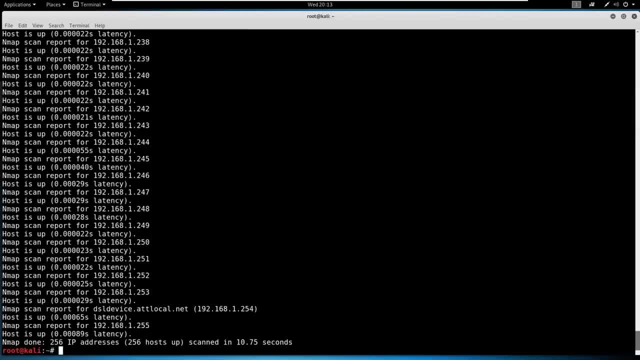 off right and um, they're going to take some time, okay. so if you look at how this looks, it says everything is up right, 242, 243. i don't have this many devices in my network. um, i do know for a fact 254 is up because 254 is my router. 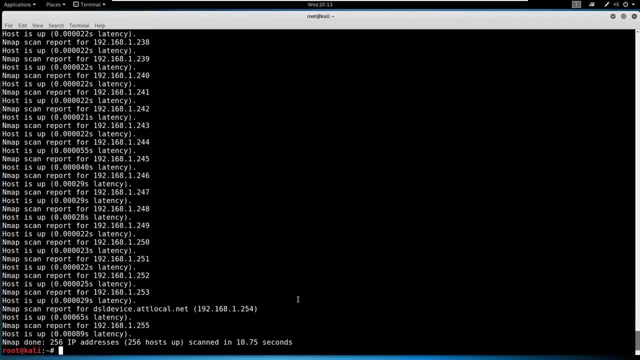 you guys can see that i'm on lovely at&t here, uh, somebody said: if you don't understand the slash 24 after my ip speak up, you are more than welcome to ask about that. if you need um, i have a video on subnetting insider notation that you you can watch. um, but the prereq to this course is some basic uh networking. 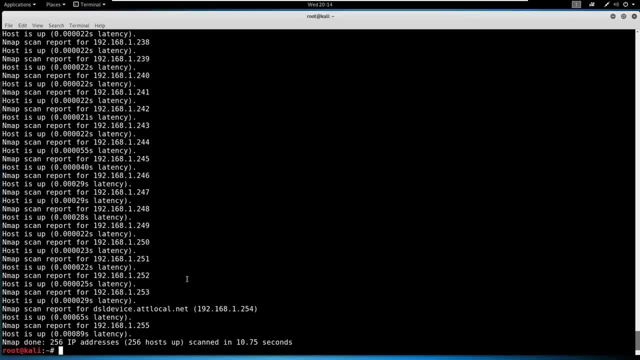 knowledge, so hopefully you all get that okay. so for the purpose of this video, i'm going to be targeting my router sitting here at 192.168.1.254, so i'm just going to run by default very, very, very basic scan. this isn't a scan that i would run normally. this is just to show a proof. 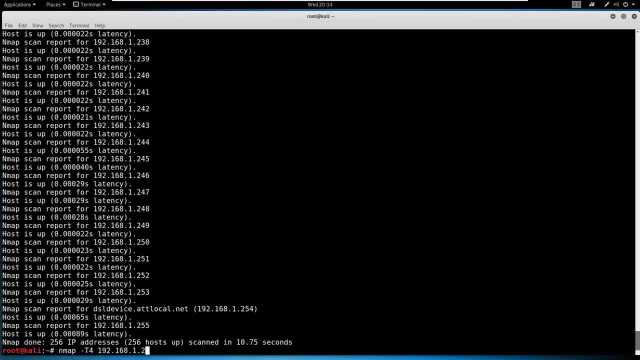 of concept. okay, so i'm running nmap, i'm running this t4 thing, and then i'm putting in an ip address. okay, i hit enter and it's going to do a scan. so i didn't put in some important information and we're going to develop and build our, our nmap scan as we go. some important information, that's. 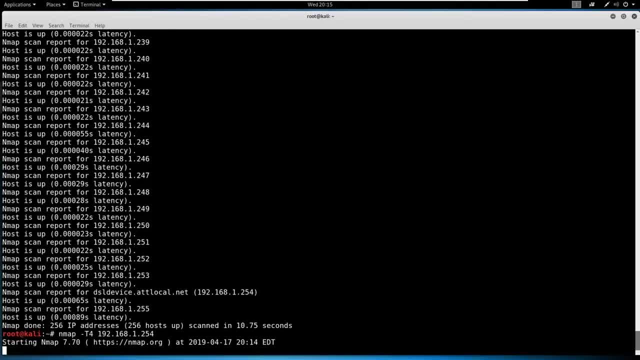 missing. well, let's talk about what's here first. so we see the t4. the t4 is a speed, so we can put t1 through t5 now. t1 is very slow, t1 is incredibly fast. the faster you scan, the more likely you are. 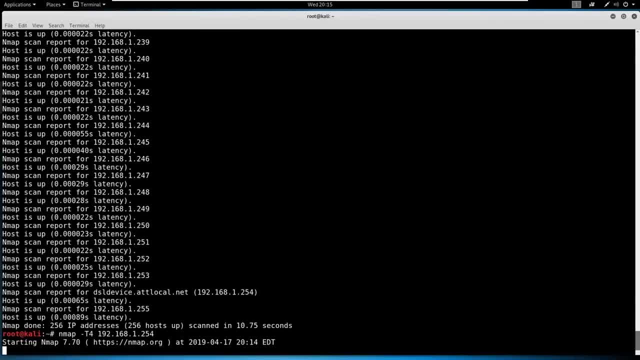 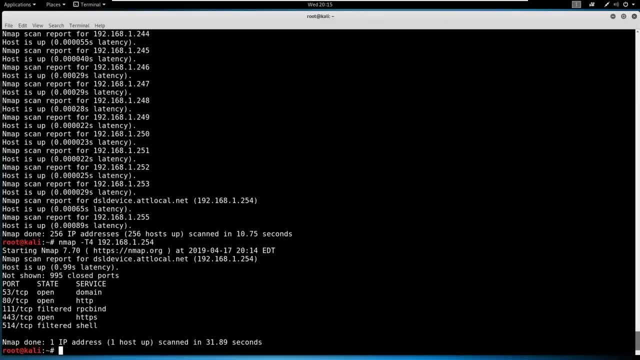 to miss something and perhaps be detected, but this isn't really the stealthiest of scanning as it is. another thing that we're going to be talking about is the speed of scan. so if you're just when you're just capacity shown at t4, you're going to click on the marsupial and 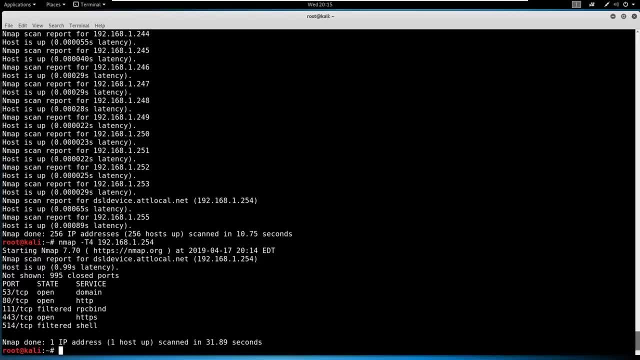 vette button and then scan in the same way. we're going to scan it in our 로드 following the sesto point, just to make sure that it's a good screen, like i do normally. this screen you want to be care for, then you want to let go of it and you want. 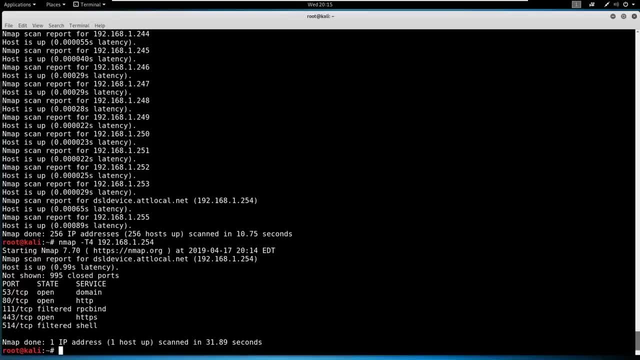 to just put in the cursor and after that i copy or paste it. i'm going to enter this as the number of cells, that x1 is, which is the number that you want. so if you load it as two gates- because that's something you're missing here- anything else you want to do? 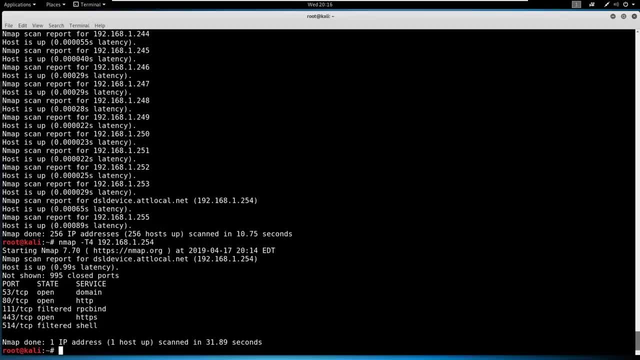 then way somebody said 65 355. thank you for that. um, so if we search the the top 1000, we're gonna miss quite a bit. what if i got an open port on this router or this machine? that's sitting at like 47 000 just as an example. if i scan the top 1000, i'm gonna miss that, so you're only hurting. 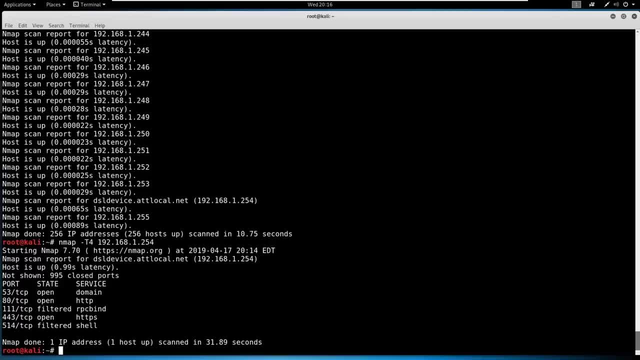 yourself if you don't scan every single port in the tcp range. so we are scanning tcp right now. we're going to be covering udp here in a minute. 65, 535 is actually the answer. okay, so what we have done is we've found at least what kind of ports are open and we can start. 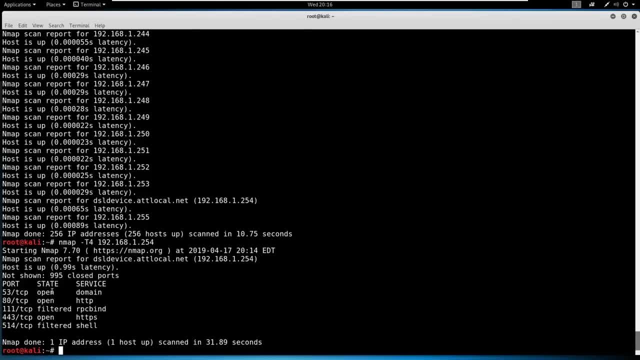 building um information here based on what we see right. well, we're running dns, okay. we're running a web server. we're running a https web server. we've got some filtered shell here and filtered rpc bind. uh, when it says filtered, you know, i'm not certain that that's actually open. it could be a false positive or it could be open, but it. 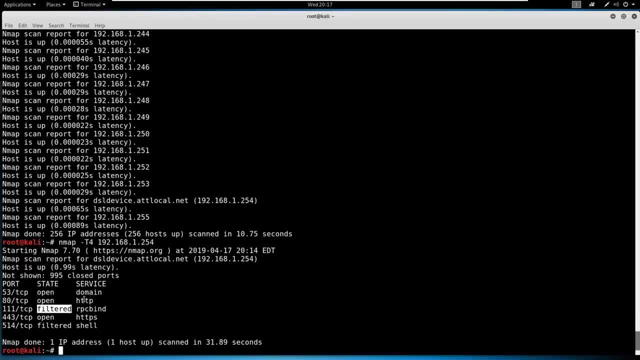 truly is filtered and we have no access to it. um, so, looking at this, i would probably want to scan this more in depth. uh, so, when we're looking at it, let's start adding some things that may, may, add depth to this. now i'm going to show you, just as a time saver, the method that i use. 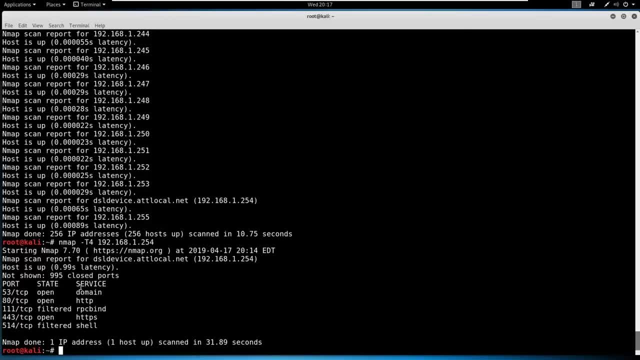 typically for hack the box or for for anything, even if i'm doing a quick scan when i'm in a network, um, this is pretty much my all-inclusive go to have memorized etc. and it's not very complicated at all. so my scan looks something like this: 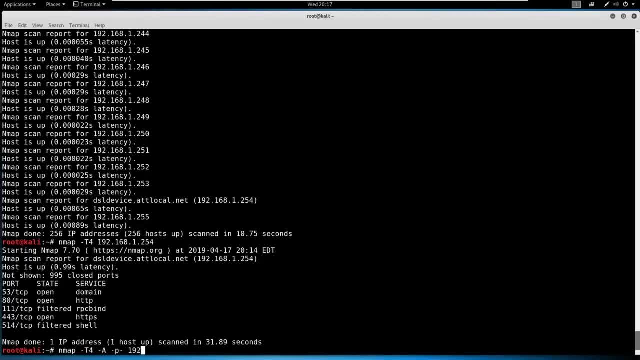 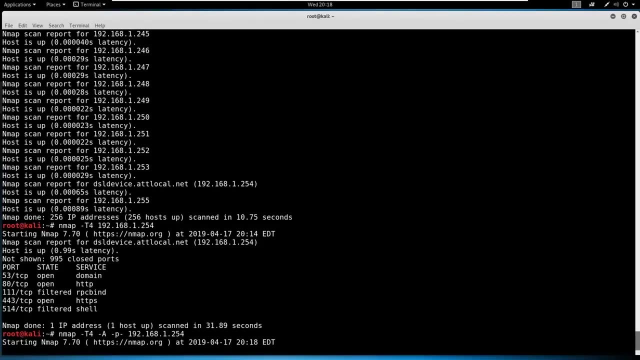 now i'm going to hit enter on this. this will take who knows how long. this could take- over an hour, depending on how long it's going to scan- and we're going to talk theories and methods here in a second on how we can improve upon this. okay, so what i'm doing here is we're doing nmap and 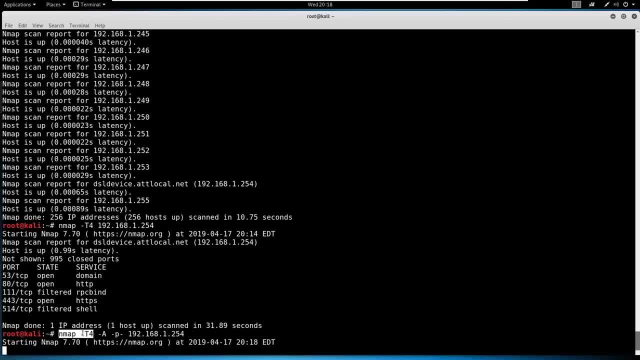 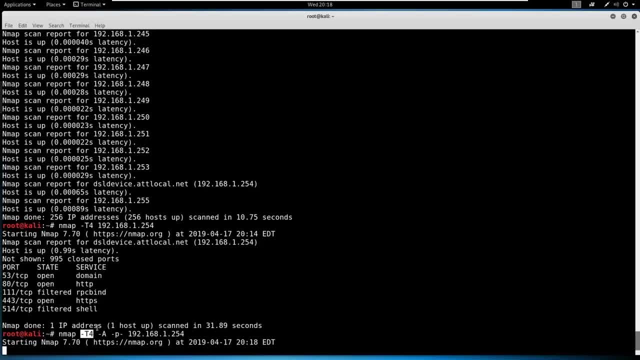 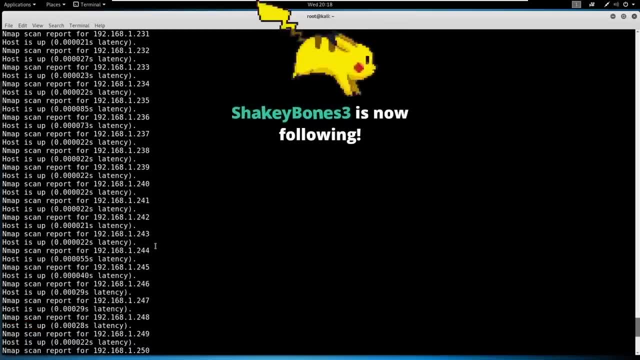 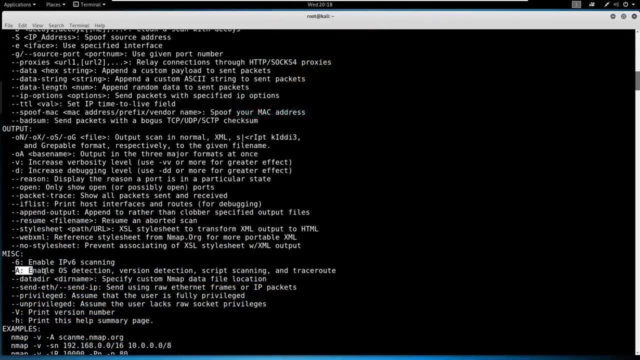 t3. i just i've learned on t4 and it seemed to work just fine for me. um, this dash a now. this dash a is for all. now, if we scroll back up through my whole list here and we go back to the dash dash, help, if you look at dash a. dash a enables os detection version detection script. 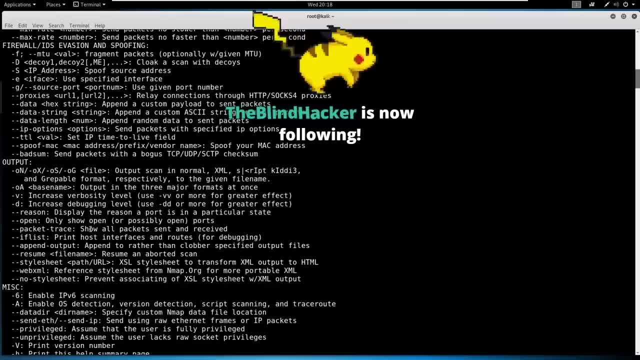 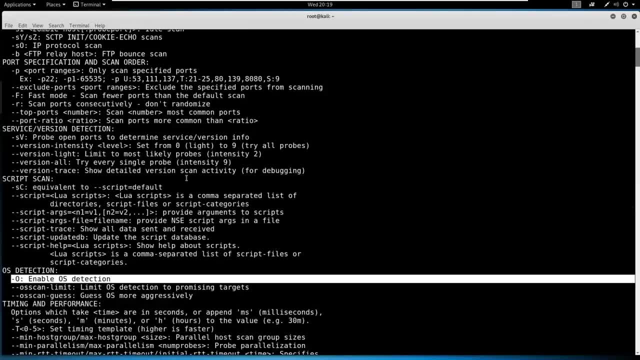 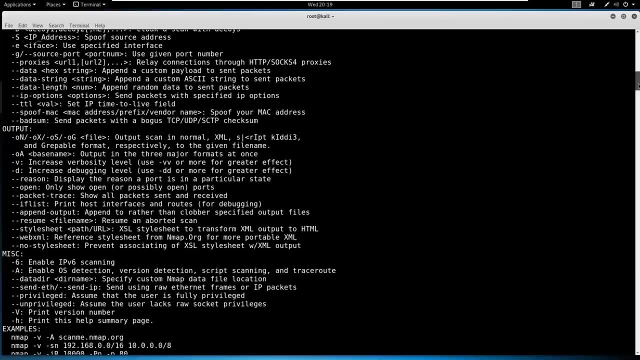 scanning and trace route. basically, what we're doing is we're doing a lot of these that are already in here, like a dash o, that's os detection, so we can aggregate a lot of what we're finding here, um into one switch of a dash a. so basically, all i'm asking for is as much information as 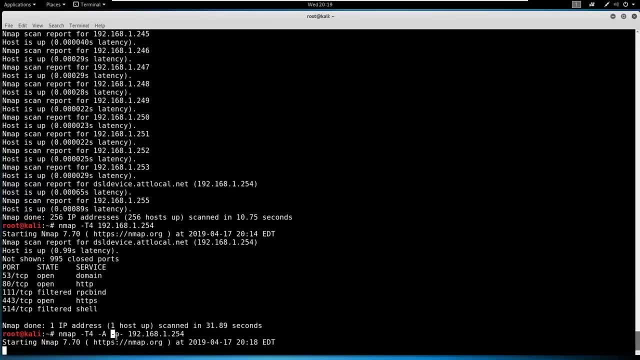 possible, and then i put in a dash p for port. but if i cap it off with another dash like this, then i'm asking for all ports. now you could write this with the dash p and then throw in a specific port, which i'll show you here in a second, but in this instance i like to scan every single. 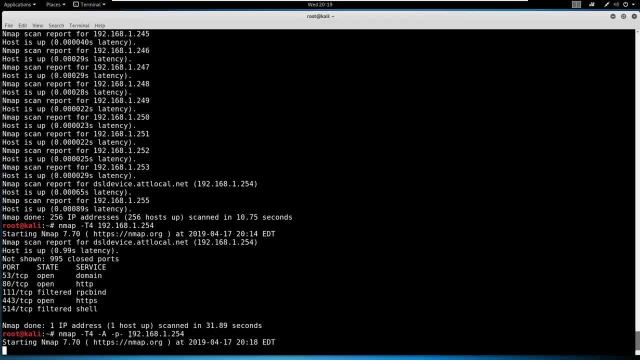 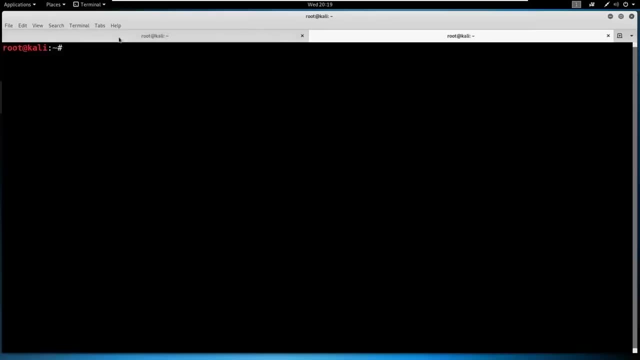 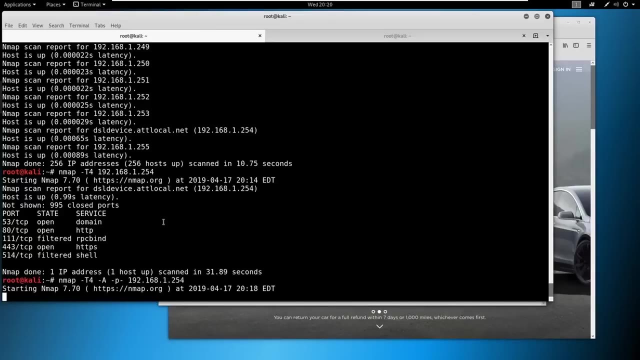 thing on tcp now and then i put in the ip address and that's what we're going to scan. let me go ahead and open up a new tab and we're going to talk theory. okay, actually, let's look at this here. so i scan this network and i scan the top 1000. 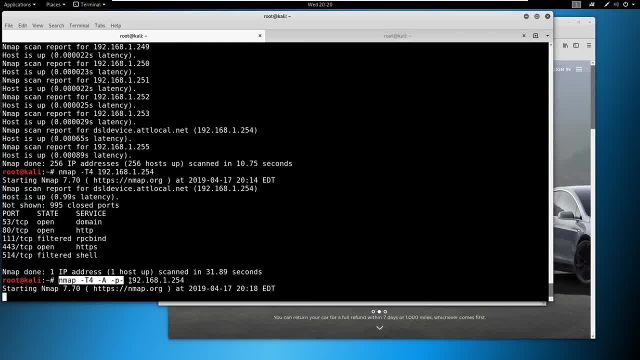 and then we came down here and i scan this network and i'm scanning intensely. this dash a is intense. right, we're doing quite a bit of heavy, heavy work here. we're doing it against all ports and we're scanning here. now what we're looking for is a way to maybe improve upon this scan and the tactic that we 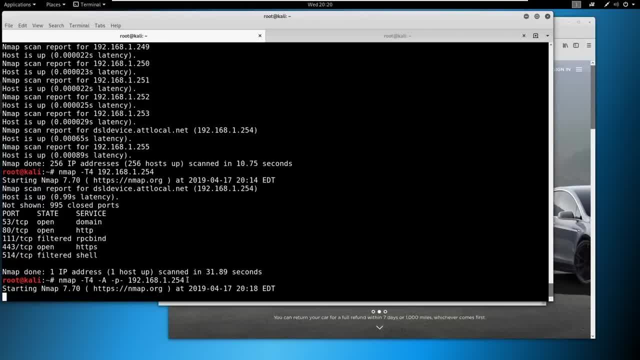 can use to improve upon this scan is something called staging. when we talk about staging, we talk about first scanning quickly and then scanning more technically, right. so i would want to do something instead of running this. let's just copy this and let's talk about how we can. 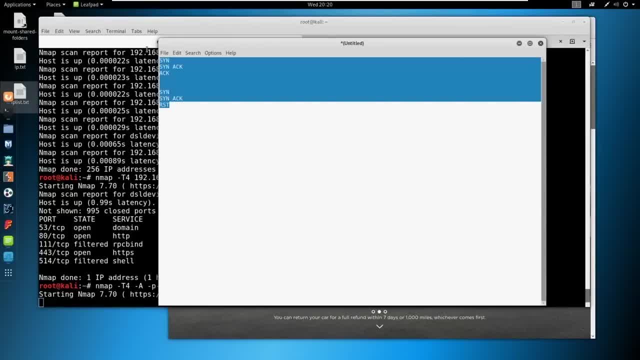 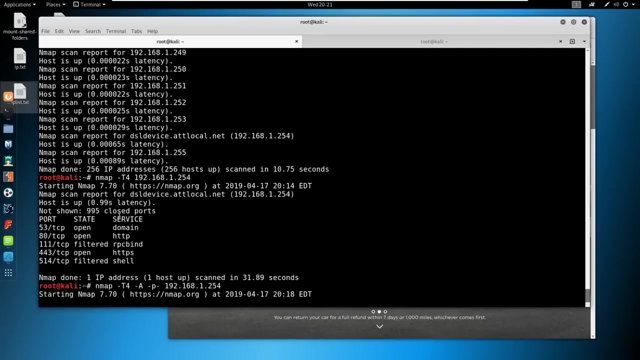 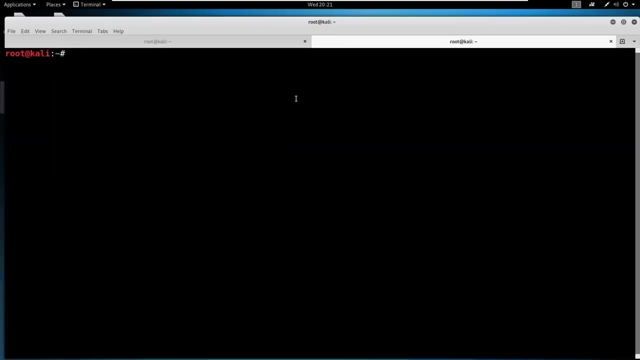 improve and we'll do a theoretical little leaf pad here instead of doing this first. what if i said: i just said mt4 ports okay. dash a is not all ports. dash p: dash is all ports version okay. dash o is os version okay. so when we come into here, and since there's some confusion from the the chat about dash, 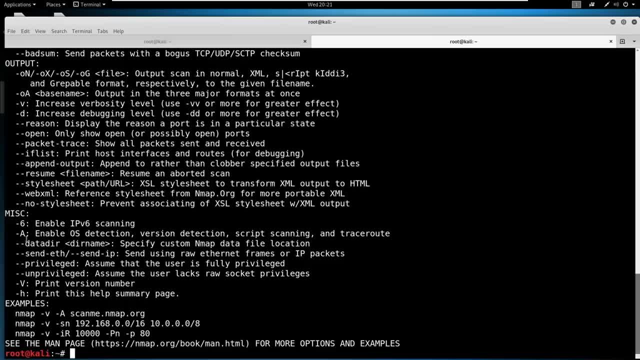 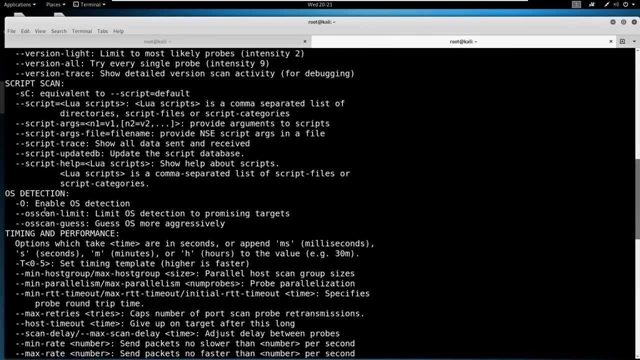 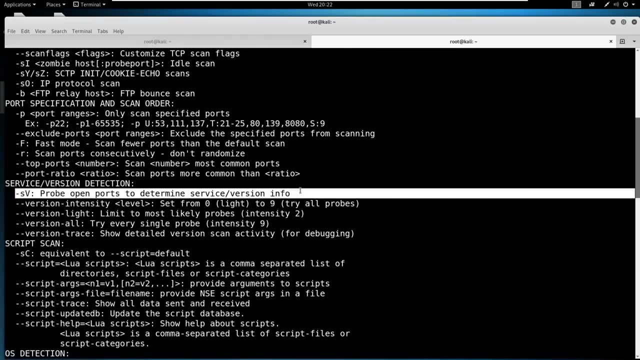 a. lets go back to help. dash a is os detection, version root detection, script scanning and traceroute. There are individual things in here. for that. There's OS detection right. Dash O Version detection is dash SV. So it kind of combines a lot of these. 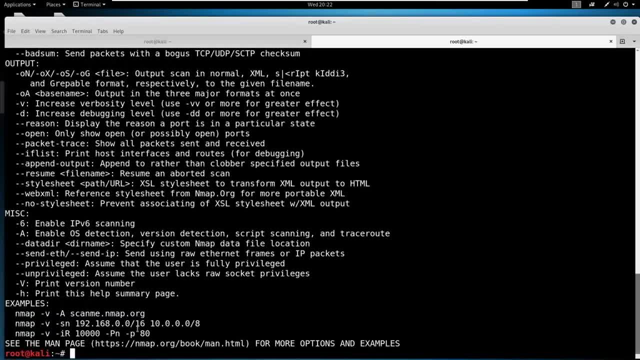 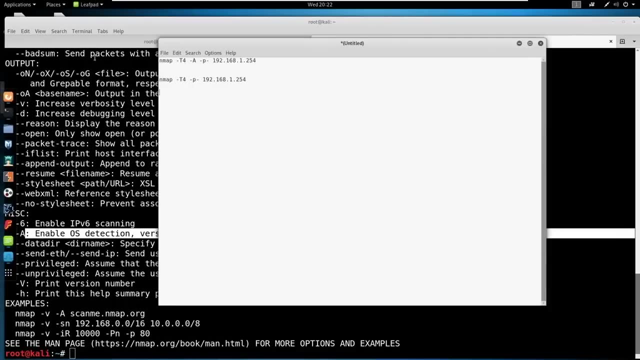 probes that you would see in some other scans. Dash A just does it all for you. Now, dash A is doing four different things at once, which is heavy lifting, And this is what we're talking about, the heavy lifting. So when we talk about staging, what if I were to scan like? so Let's. 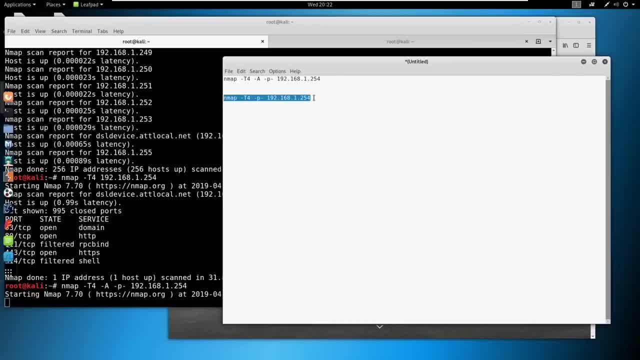 say, I scanned with this syntax right. I scanned the dash P dash, I scanned all ports, the T4, but I didn't include this dash A, So it's not as intensive. Well, let's say, let's just copy this: 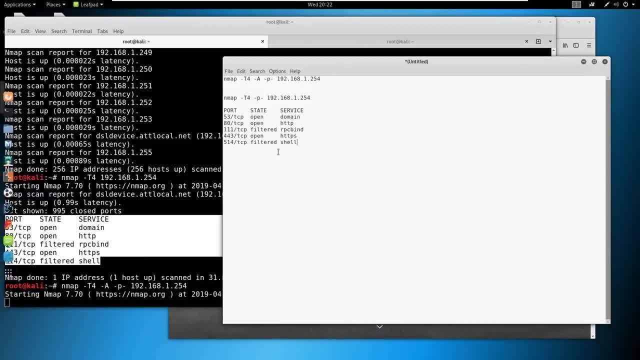 here. Let's say that it returned this scan. here We see these ports. Okay, So if I come into here and I want to get a detailed scan, it would make a lot more sense to me that, instead of putting the ports here, of all ports, and 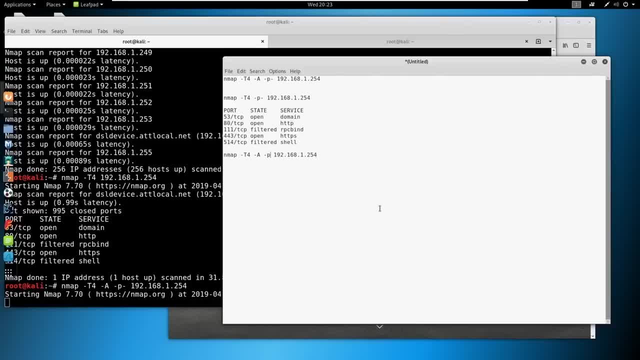 scanning every port within depth. you'd want to stage it out right, So instead maybe 53,, 80,, 111, 443, 514.. So if we scan everything, it's going to take a lot of time. If we scan the five ports that we 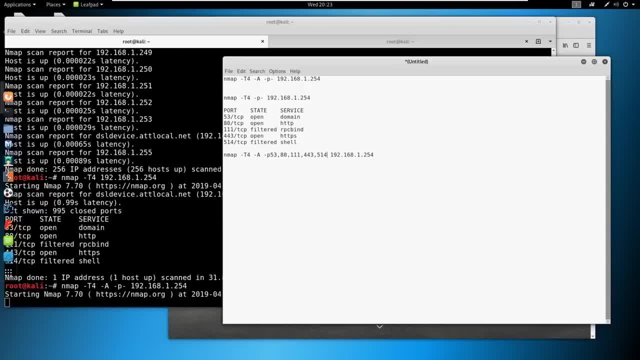 found open, it's going to take significantly less time. So if you're working on like a capture the flag or you're working hack the box, you're doing some sort of a race against the time. This is probably the go to Now. I will admit to you that I often come through here and I just run. this really quickly And I'm going to do a little bit of a test here. So if I go to the screen, I'm going to do a quick run of this scan. So if you're running a scan, you're going to do a. quick run of this scan. So if I go to the screen, I'm going to do a quick run of this scan. So if I go to the screen, I'm going to do a quick run of this scan. So if I go to the screen, I'm going to. 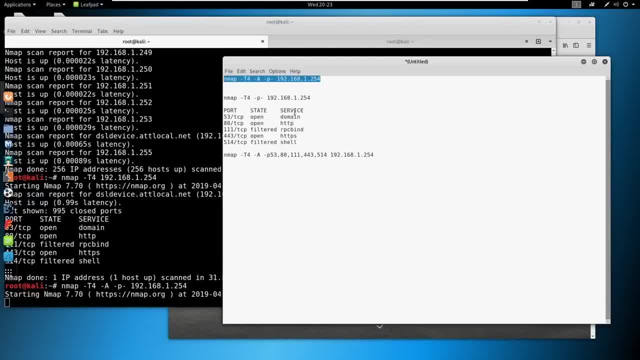 running a scan. There's nothing wrong with this, It's just tedious. Now, for those of you who are overachievers, we can make this even better. We could do something along the lines of taking this right And we'll come down here. And what if we put it into an output of all and you just say: 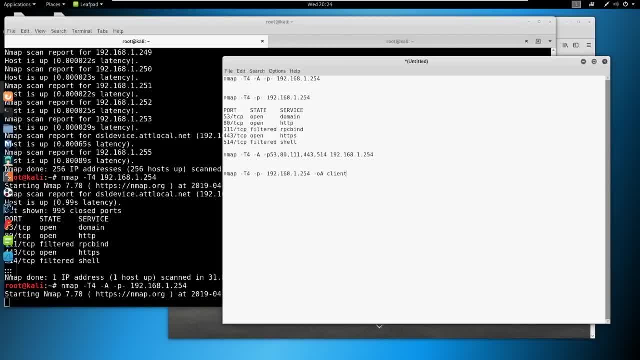 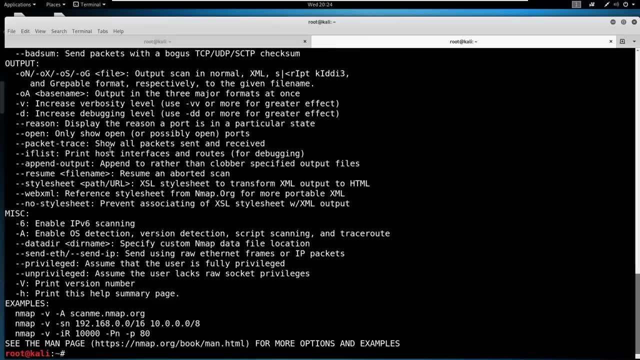 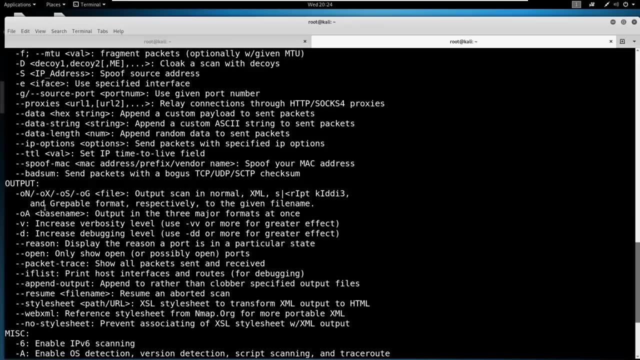 whatever, you just give it a name of client, Right? So it'll give you a clienttxt, a clientxml. Let's see what the output all gives you. It gives you the three majors, So a txt, an XML and a ScriptKitty and grappable format. 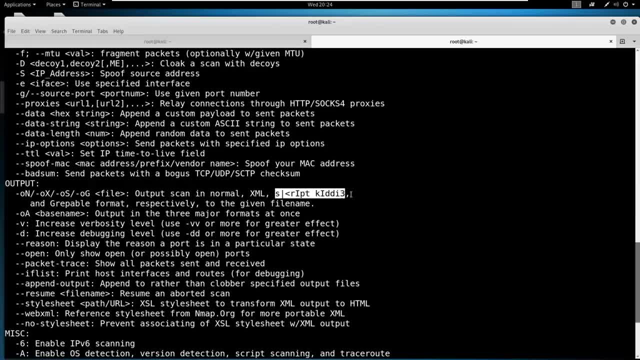 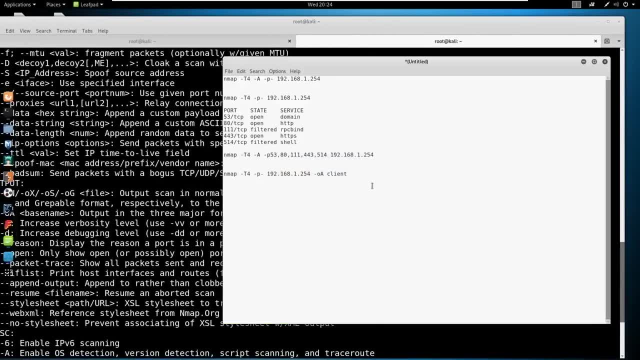 So it gives you four. it looks like. Well, it says three major. I don't think the ScriptKitty is a major one. Okay, so it gives you those three, right, And you can take these results. Now that they're stored again, they come out and they come into these files. 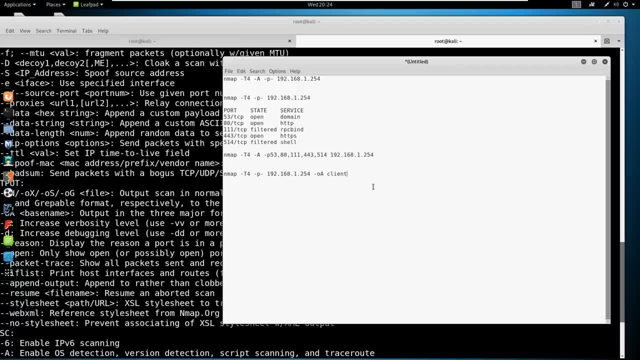 Now you could build something that says: okay, we'll find the results that come out of this scan, in particular looking for this client name or whatever we entered in here. It could be a $1 for a variable or an entry right that we talked about in previous weeks. 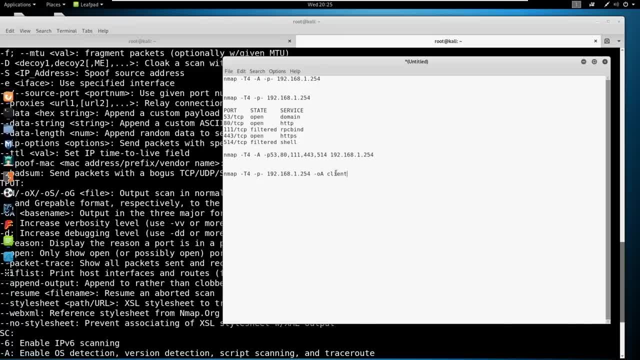 You could take that logic and you can say: grep through a file, search through a file for all open ports that you found and then append those into this list here And then search. So you could do your own staging script to make this work. 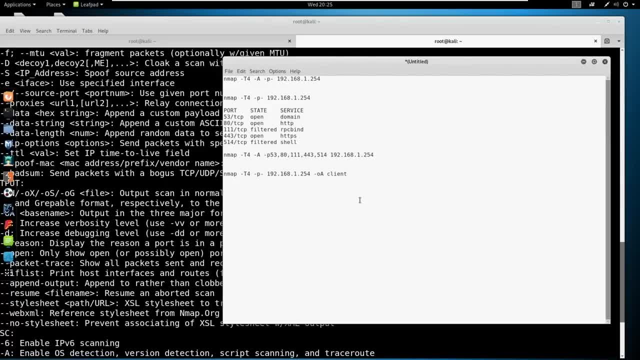 These are just some advanced thoughts. We're not going to get into that today, but these are things you should be thinking about is how to stage, how to improve in ways that you can just do things a little bit faster. So in my job we have something that was built before my time. 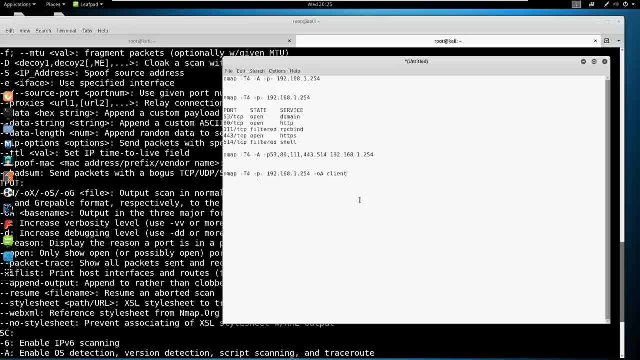 but basically it doesn't. So we have something similar to this and then it goes out and it runs a bunch of if statements, right. So say, for example, it says: if port 80 is open, I want to run Nikto scans on it. 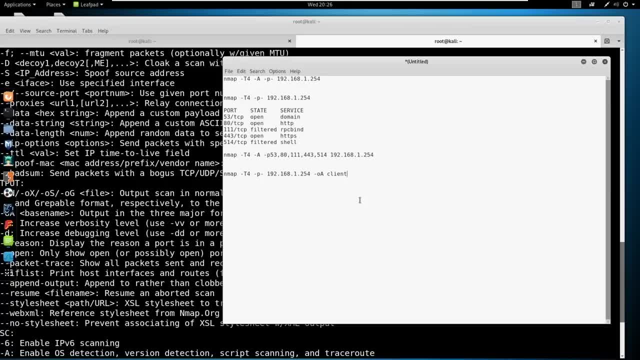 I might run some kind of Durr Buster or Durr on it And we'll talk about those tools here in a little bit. But you can start adding and chaining more, and more and more and build out these scripts to where you're letting it do all the work for you. 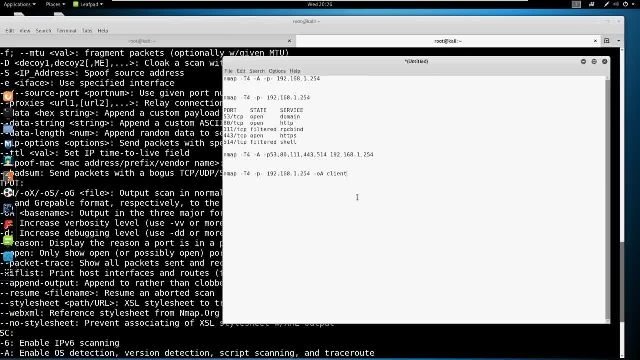 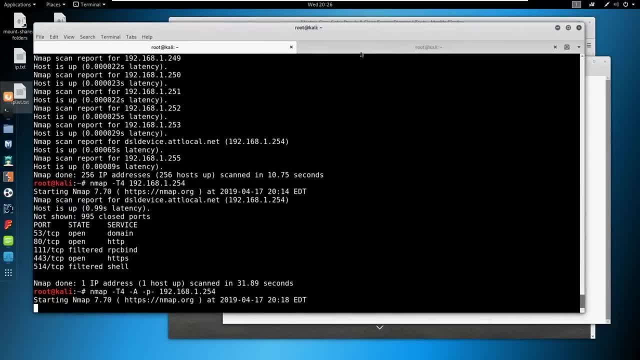 This is where scripts, This is where scripting becomes super powerful. So food for thought. We're going to move on. Okay, so you can pretty much hit any button. I typically hit the up arrow when I want to check on my scan. 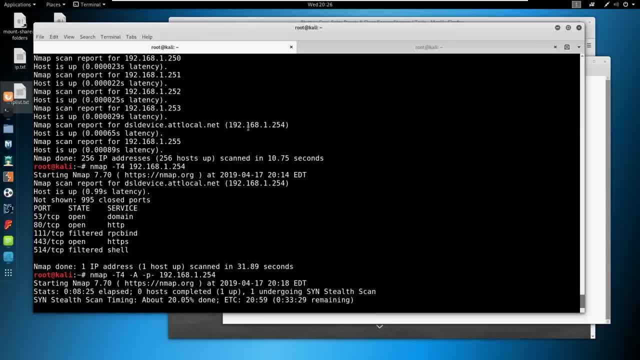 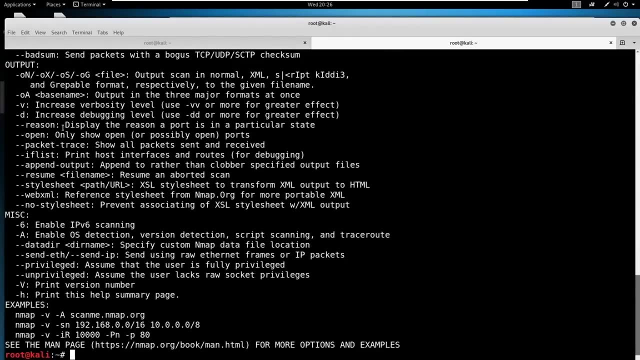 It says we've got 33 minutes remaining. We'll see how long that actually is. You could also do a dash V for verbose, and there's a status update every so many minutes- one in here as well. I forget what that one is. 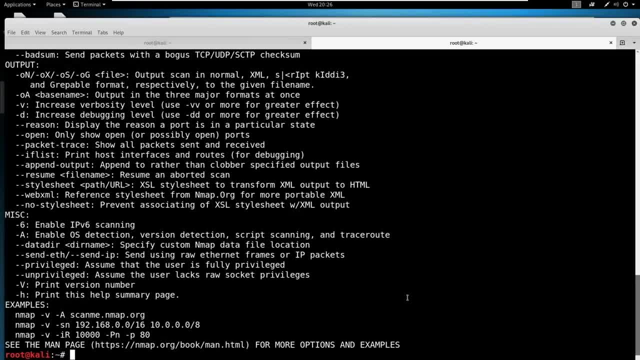 I never use those. So the question is: from Sick in the Mind that you've got a script that's similar to this and you want to share it. You're absolutely welcome to share it. Save it for me too, and I'll share it in Discord if you don't mind. 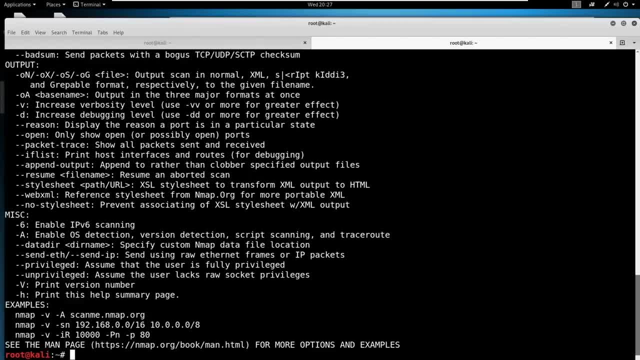 Okay, I'm going to take a drink real quick. What kind of drink? I've got a monster, because I'm tired, I don't sleep, Okay, So we've talked about scanning the TCP side of the house. Question came in. 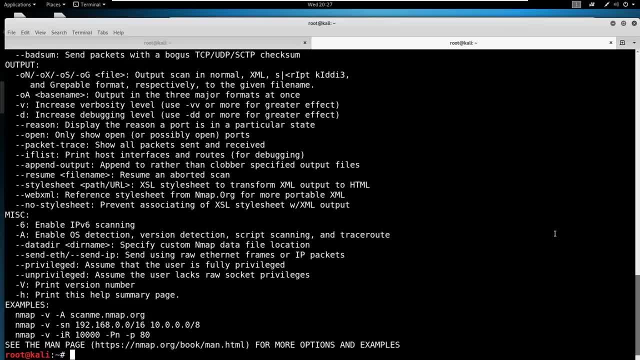 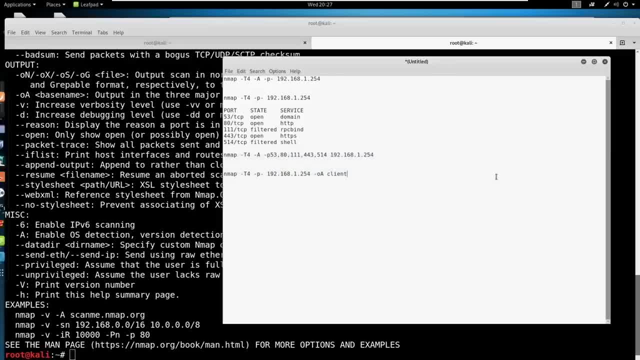 And I'm going to say dash A dash P dash, And I'm going to say dash A dash P dash And I'm going to say just dash P dash. Okay, So dash A is the all. It's the intense scanning right. 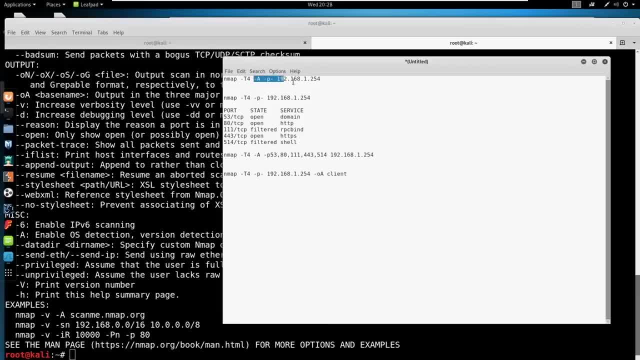 We're intense scanning all ports, So 65,000 ports here. We don't know if they're open or they're not open. Now, when we're just scanning the dash, P, dash, we're not doing it intensely. This will be much quicker because we're not doing the dash A. 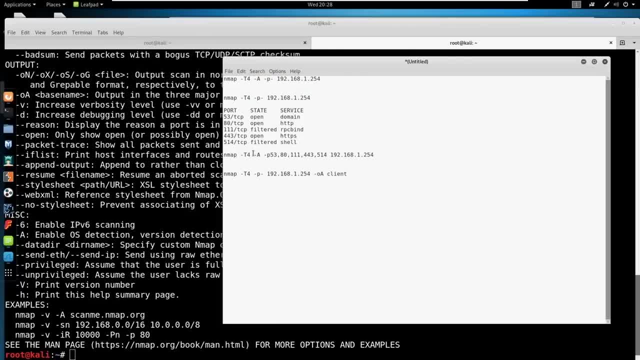 The dash A takes a lot more time. So that's where the theory comes in that dash A on a few ports that you find, as opposed to a bunch of ports at once, will save you quite a bit of time. The dash A affects everything you tell it to scan. 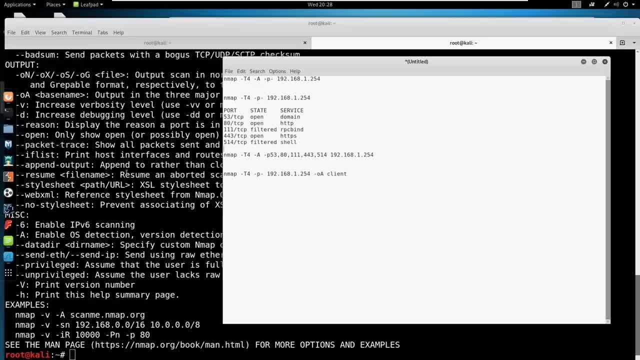 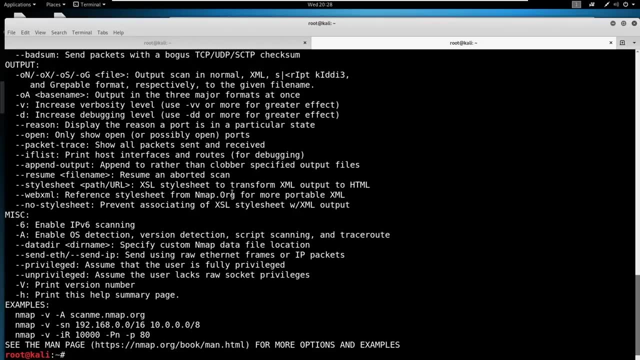 The question is: does the dash A affect all ports? It affects everything. you tell it to scan. All right, a little sidetracked here. So let's talk about scanning with UDP here. So you've seen the dash SS, We don't have to use it anymore. 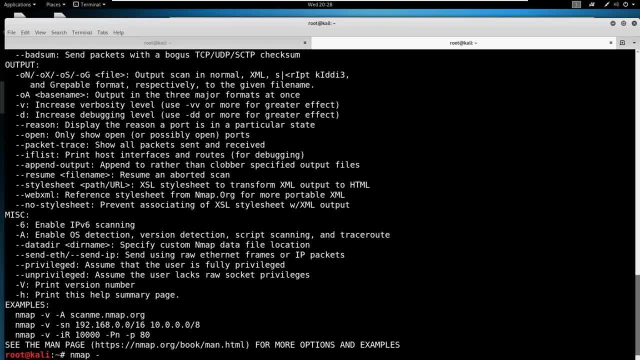 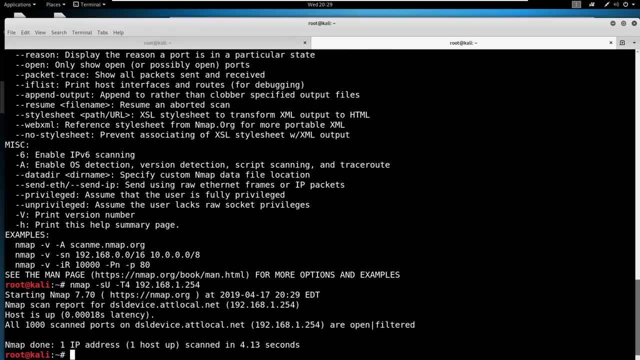 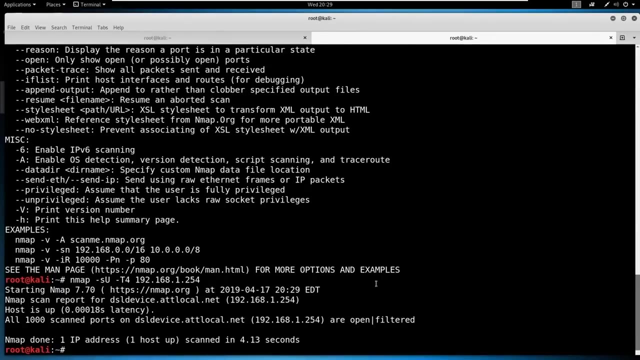 So if you wanted to scan a UDP, the syntax looks something like this, at least in my case, And you could pretty much hit enter. here I never use T5, never, Okay, Okay. So UDP is highly unreliable. UDP takes forever, as somebody already said. 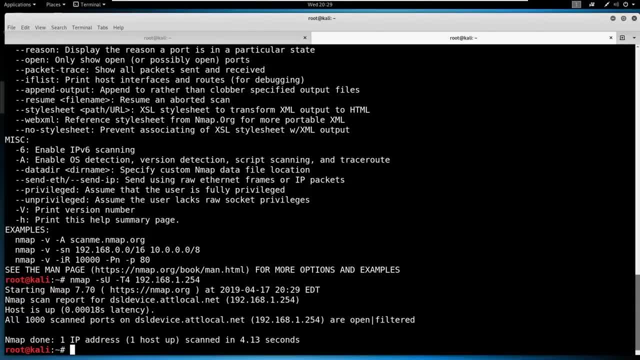 And there's a big reason behind my syntax here. I did not include the top or I only included the top 1,000 ports. As you can see, it said we scanned 1,000 ports. If we were to try to scan 65,000 ports on UDP. 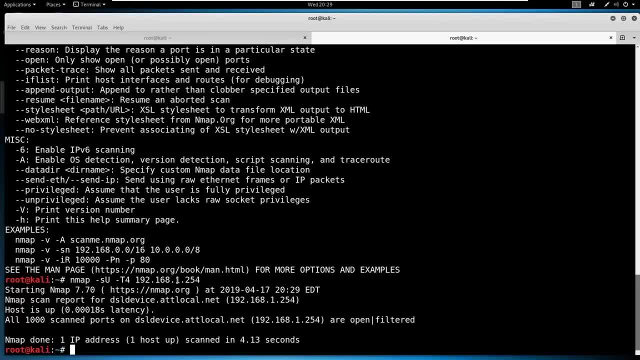 it would take hours, Just hours. So also there's a lot of false positives that come up. You really can't trust a UDP scan. Not to say that UDP scans are not important. You can find some interesting information on that side. 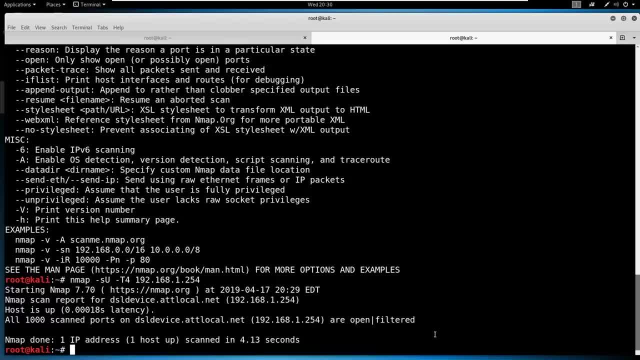 But typically they're hard to trust right And they're time-consuming. Basically, when I'm doing scanning, I let Nessus try to find that. If Nessus doesn't find it, then so be it. We can find interesting information. 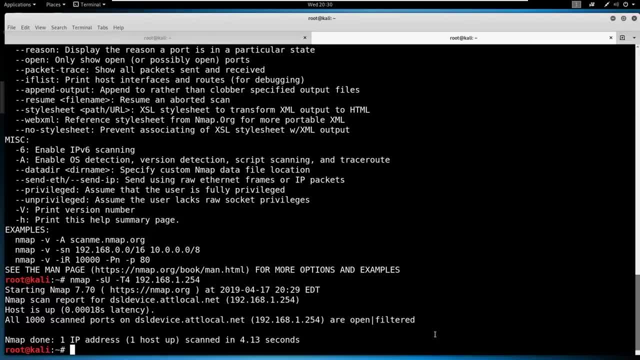 like SNMP and have a public community string- things like that. that can become really fun if we can find some things on UDP. Just know that 95% of your work is going to be on TCP. However, if you're taking something like the OSCP, 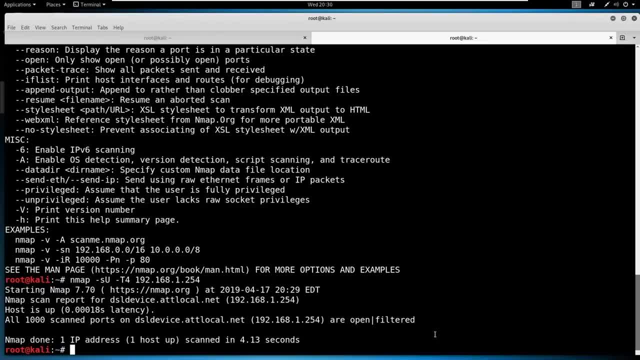 or you're doing Hack the Box or even real-life environment. you should not neglect UDP, because there will be something there And if you miss it, you're going to miss it. So just know to look under all the stones. 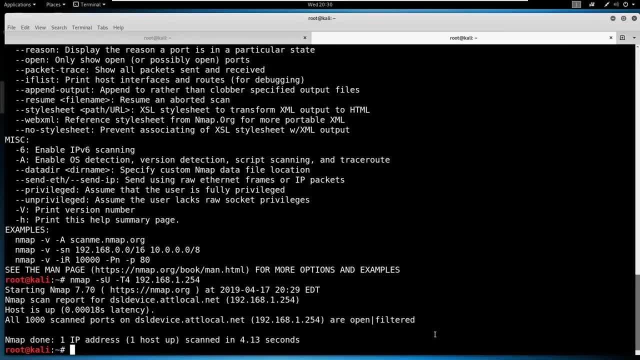 Don't just focus every time on TCP, or you're going to miss things. All right, other than that, one more thing with Nmap I want to show you. then we're going to move on. So if we ls user-share-nmap-scripts. 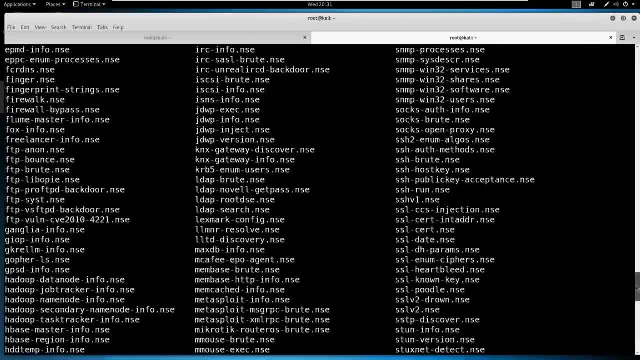 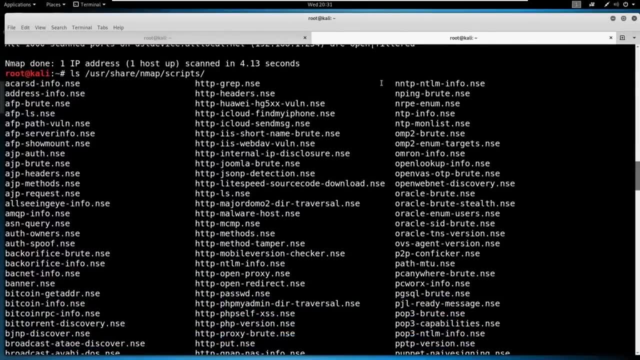 Now, this is all the scripts that are available to us via Nmap. We have a script feature that I'm going to show you. We can pick any one of these scripts or we can do a dash-all for these as well to try to do some vulnerability scanning. 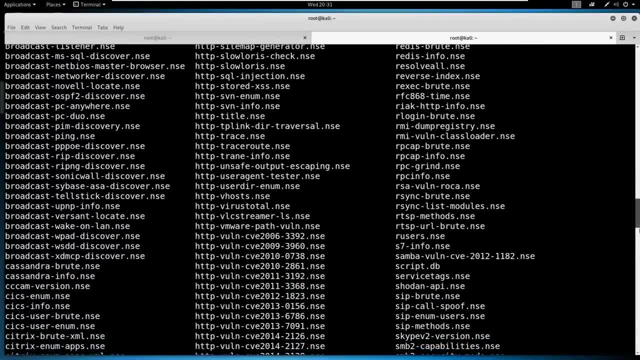 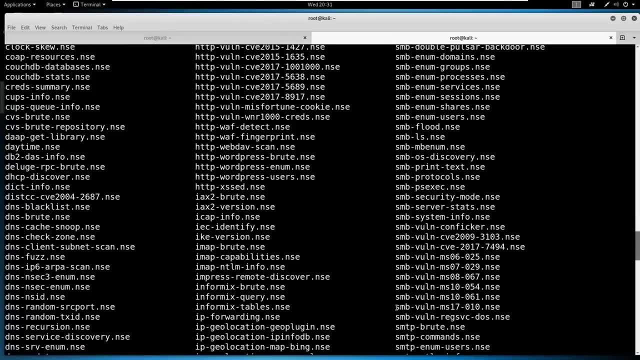 Some really cool stuff in here If you look through it. I use some of these from time to time. There's one that I really like to use and I'm going to show you. But say, for example, you think that there is EternalBlue running on a computer. 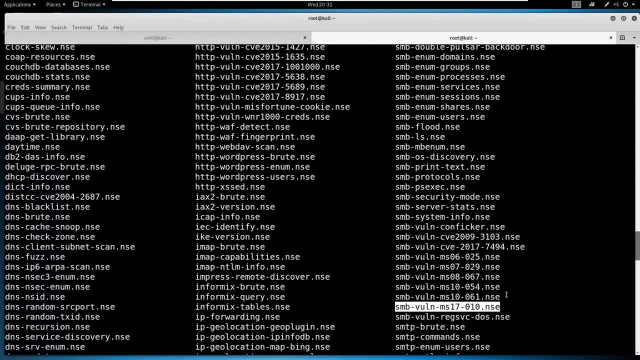 You see a window and it's a Windows 7 machine. It's got SMB. You have a hunch, right. You have a hunch that EternalBlue is running, And if you don't know what EternalBlue is, that's fine. 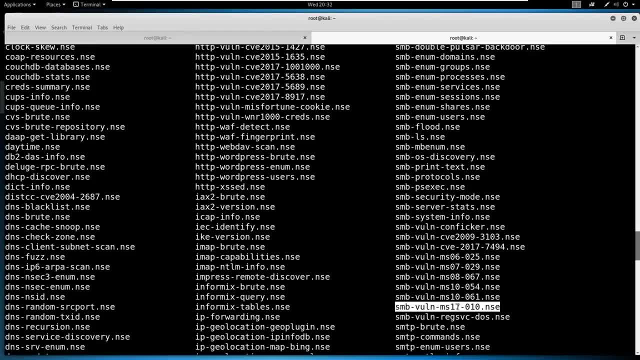 Just say you have a hunch on a vulnerability. This vulnerability, specifically, is MS17-010. And you want to know if the machine is vulnerable. if it thinks it is, You can grab this script and try to run it and see what Nmap thinks. 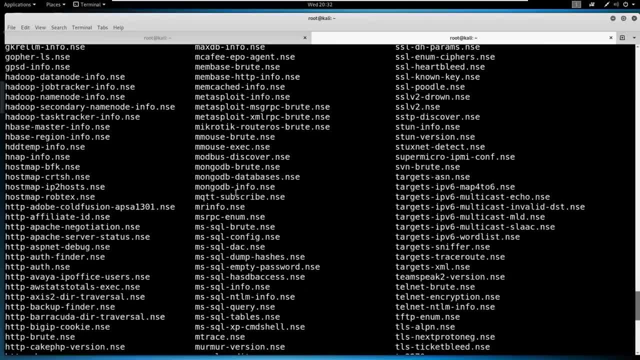 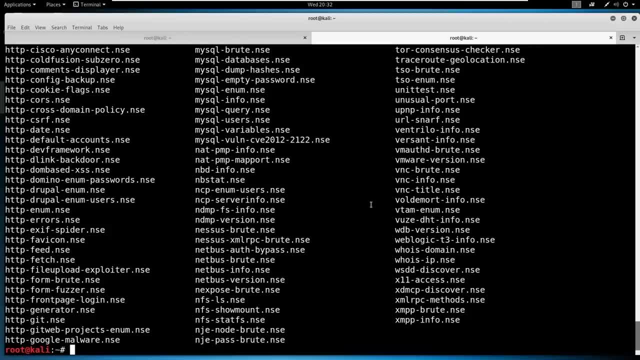 There's quite a few things. if you just scroll through here, I couldn't tell you what 90% of them do, but a quick Google on something in here might help you, And that's where it's going to come into enumeration. 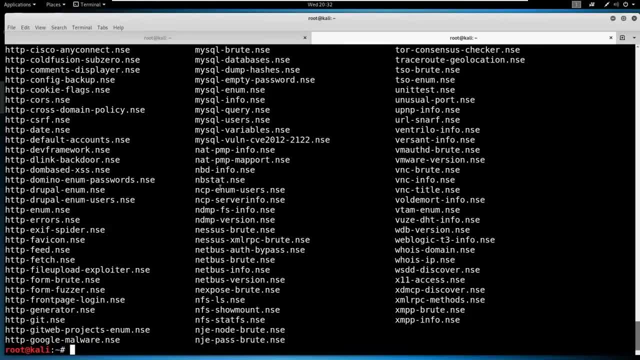 We're going to talk about enumeration next week And this becomes way, way more important. So we're going to use one script just for the fun of it, And this is a script that I use on pretty much every web app: assessment. The path is user share and map scripts. 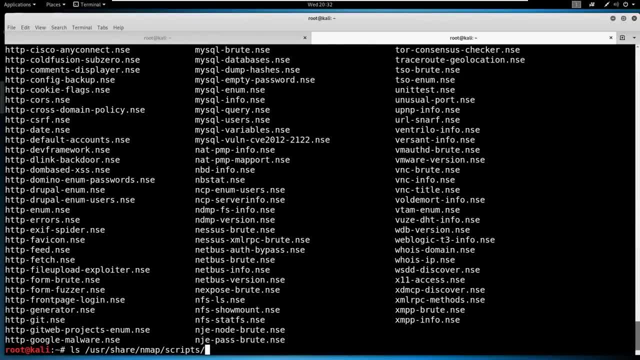 I don't know what voldemortinfonsc is. You can check that out and let us know. Enumeration is the most important thing you'll ever need in your hacking career. If you cannot enumerate, you will not be successful as a penetration tester. 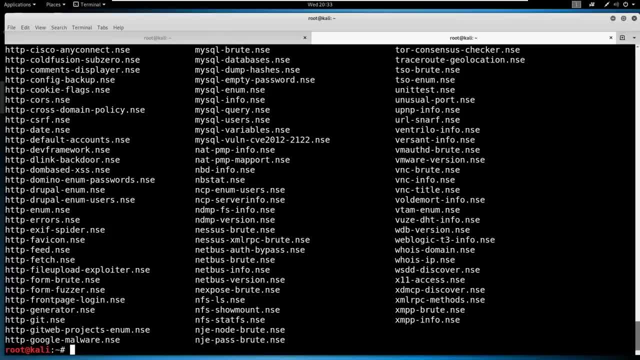 It just comes down to that, Honestly boils down to that People want to jump right into the exploitation, but if you cannot do the research, you cannot look around, you're going to have a lot of problems. All right, So let's use one of my favorite scripts. 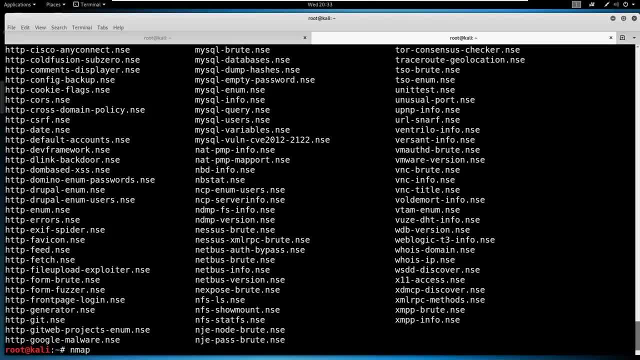 So I like to check for ciphers. When I'm doing a web page assessment, I like to see what kind of ciphers they're running. Typically, you're not going to find anything that's going to be super exploitable. Most of the cipher exploitations. 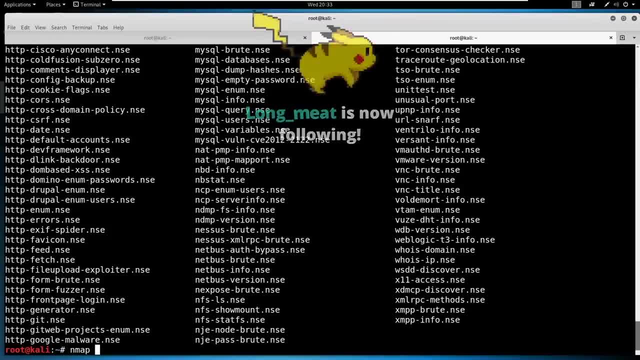 require some sort of man-in-the-middle attack. You're not going to get that lucky, but it's good for reporting, right. So what we can do is we can scan and let's just look at, let's do port 443.. 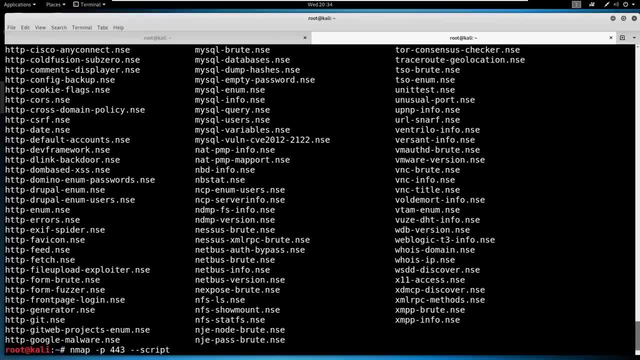 And the script is: we just do dash dash script like this. We could say equals. Now if we wanted to run all scripts against a host- and I do not recommend doing this against the host we're about to use, but you can do it on your own. 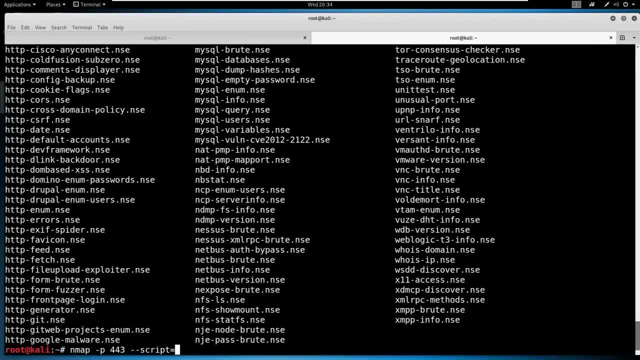 or against a hack, the box or a vulnerable hub. if you want, You can do equals all. It'll run all the scripts in that folder. That'll be some time time consumption. The one I like to use in particular is SSL enum ciphers, just like that. 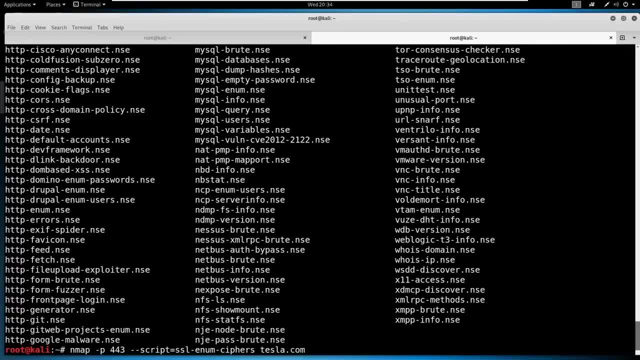 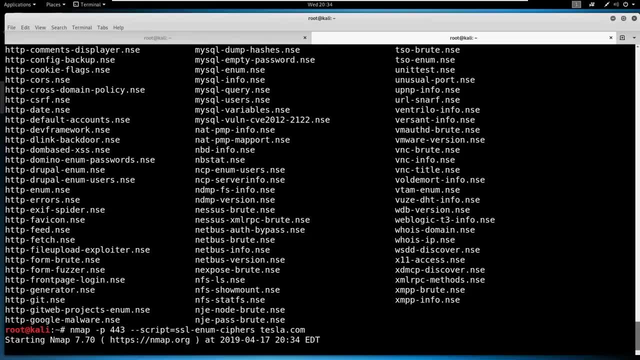 And we're going to go ahead and just say teslacom, Hit enter. This is going to sit here in scan: teslacom for all the ciphers. What it's going to look for is all the ciphers it has. it's going to give you a rating on all the ciphers. 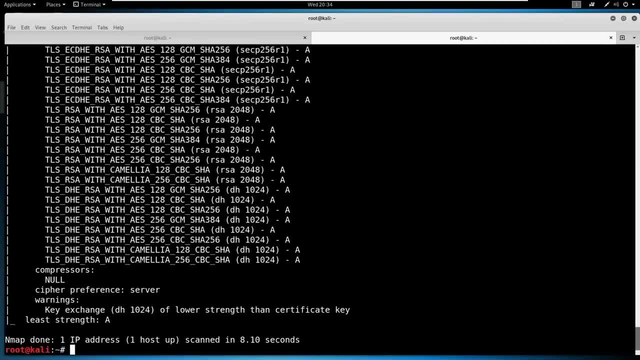 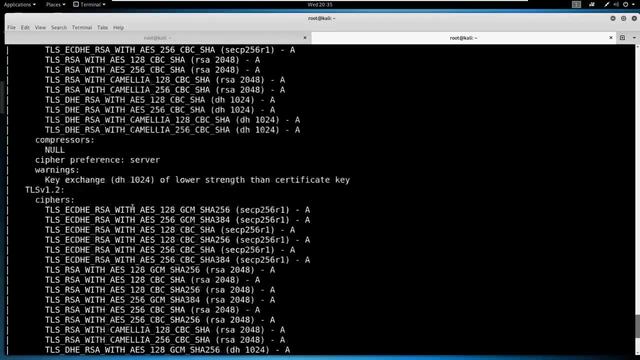 and then it's going to give you the least strength of a cipher. If you look at this, you can see that Tesla does a very, very good job of keeping their ciphers up to date, And it shows what returns back on all of these. 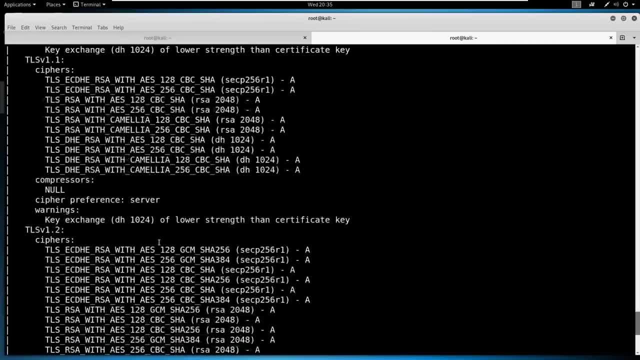 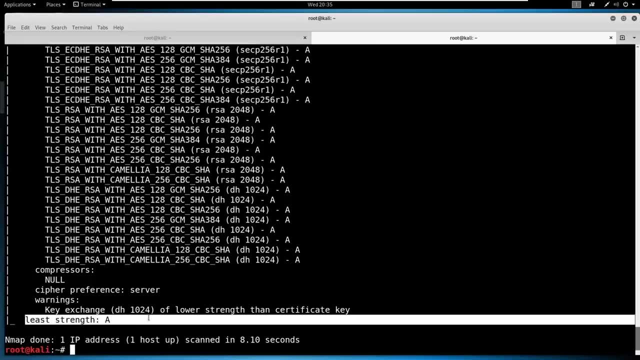 So everything looks like it's TLS. It's got all the different types of ciphers And the key of least strength here. I mean we're still dealing with an A. So very, very impressive on their behalf. Usually you see something in there that's a C or a D. 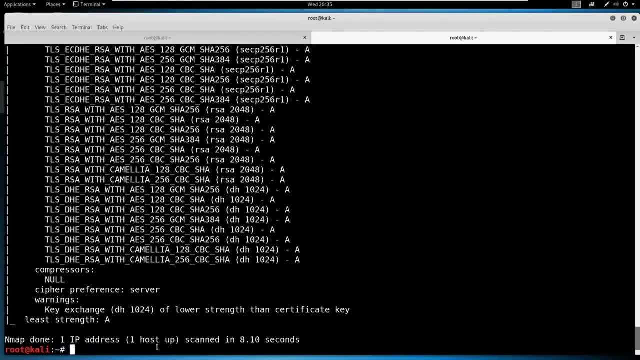 for a lot of websites that you look at. So, but yeah, that's scripts. There's also tools on the web that can do this, but just know that Nmap is fully capable of doing a lot of things that you can go do out on the web. 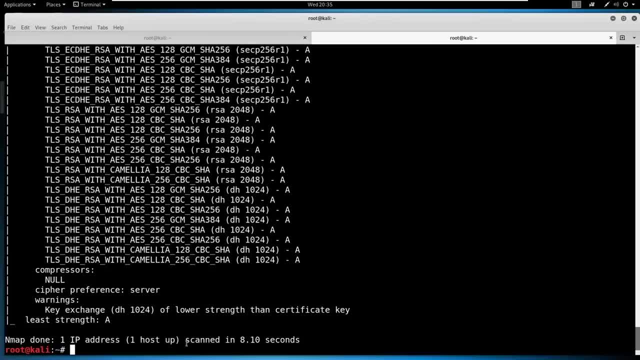 All right, that is all I have for Nmap. We're going to move into other products. now Let's go ahead and download Nessus. We're going to need to spend some time with Nessus and get that running. That way we can do a scan. 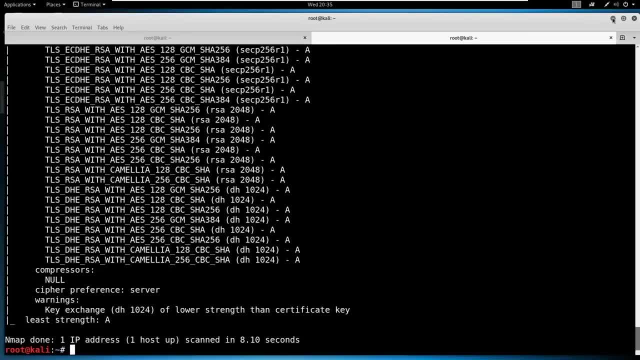 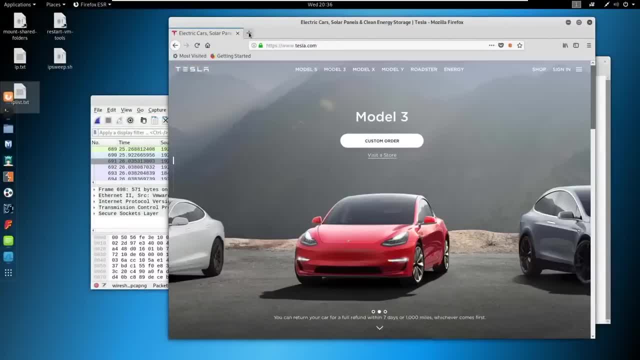 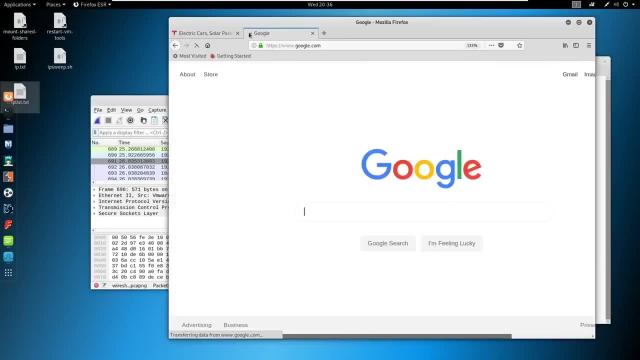 and work on some other tools as well, So I have intentionally not downloaded Nessus on this machine. Let's go ahead and go out to the website here. I'm just going to go Google and then Nessus Home. There's a free home version out there. 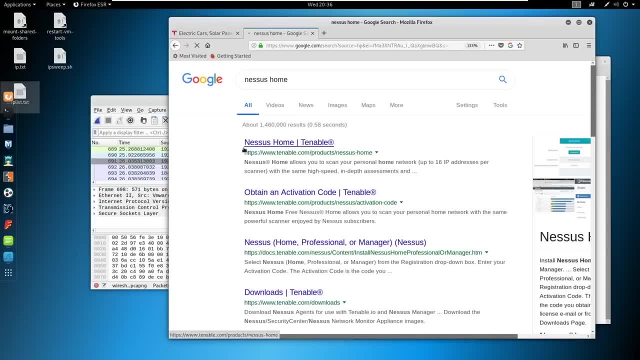 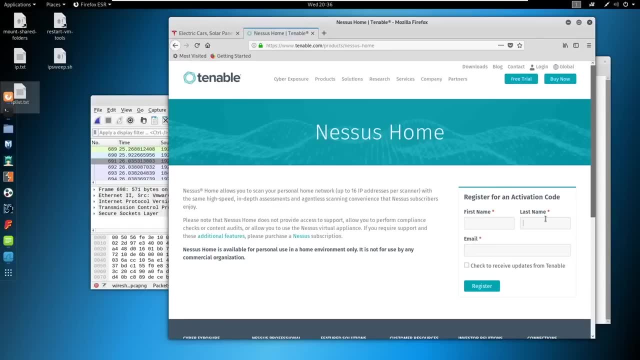 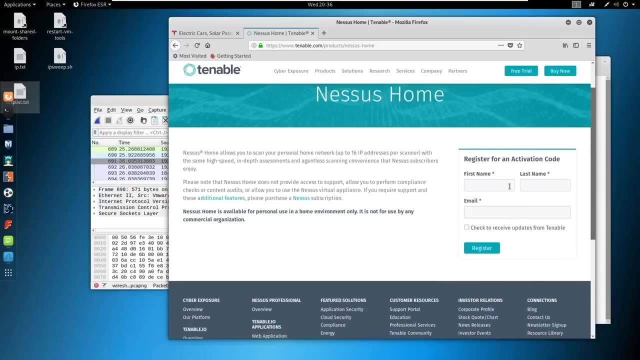 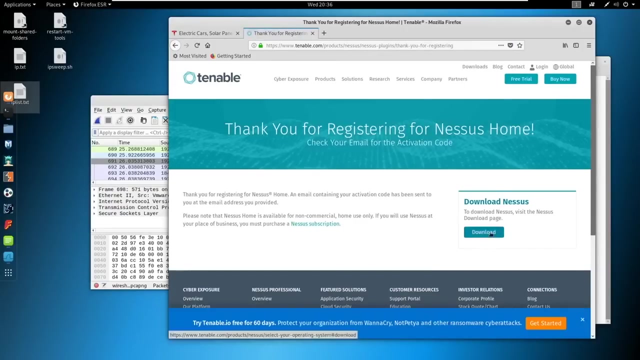 Now you do need to put in your name- first name, last name, email address to register. I'm going to use random stuff here, because I have an activation code somewhere floating around here. Just register. Once you register, it'll give you the option to go to the download page. 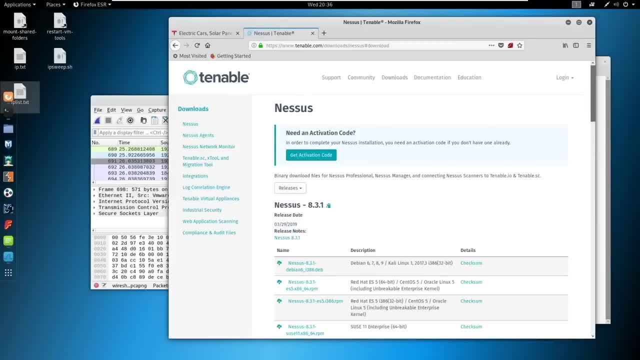 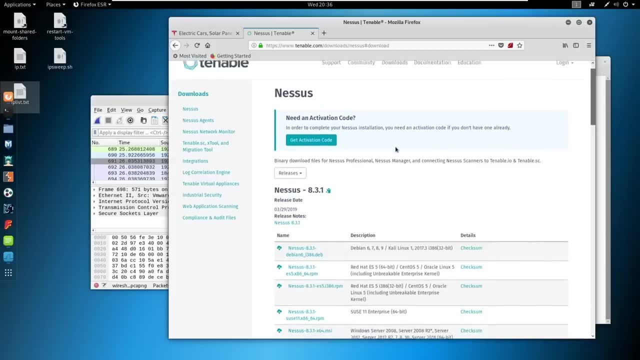 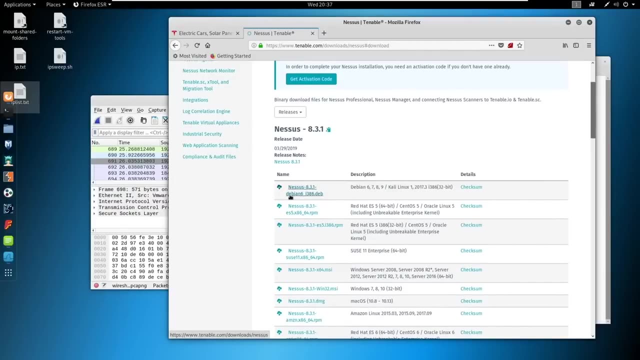 Go ahead and click download. I need to grab my key real quick while we're talking, All right. so what we're doing is we need to download. We're using Debian right, Debian Kali, So we're going to download our Debian file here. 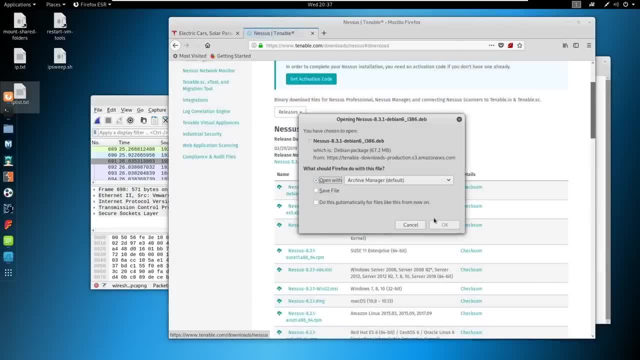 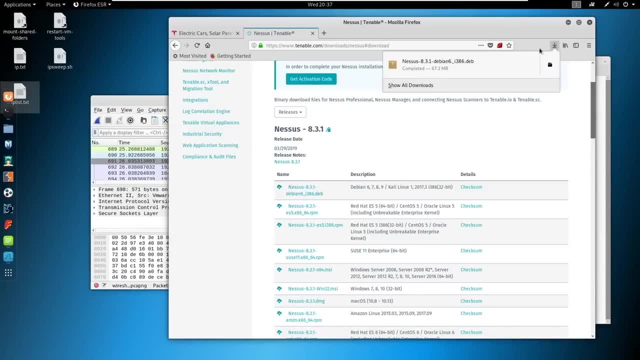 Just click on this button. Agree to their terms. Save the file. Let that download. Some of you may have slower connections, so I'll give you a minute, And then I'm going to pull up my key as well. Uno momento, por favor. 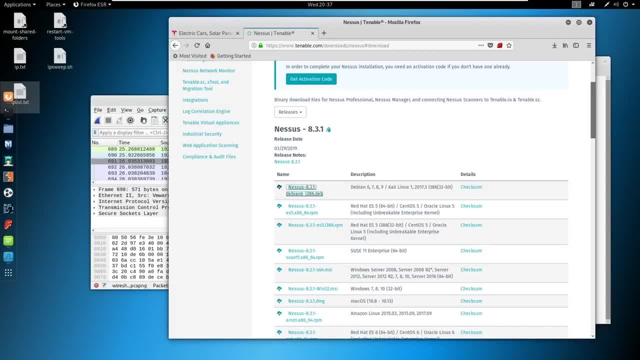 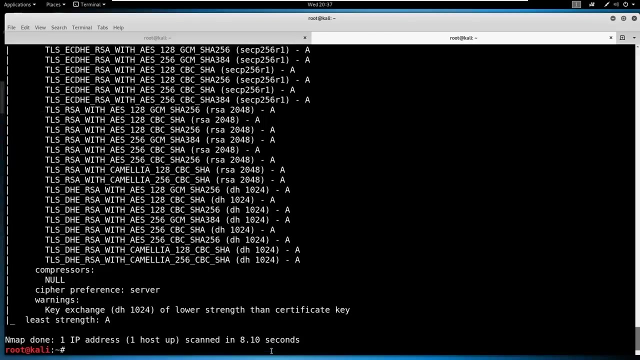 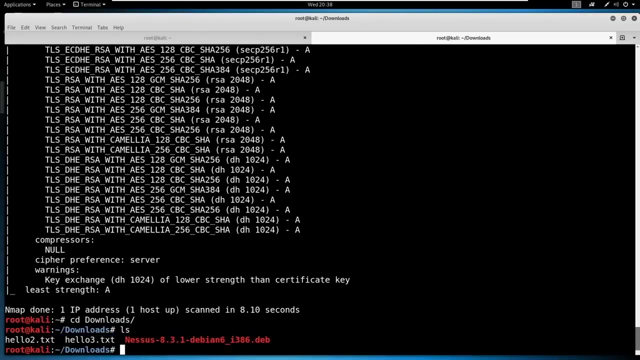 Here. Uno momento por favor. Uno momento por favor. Uno momento por favor. Okay, so let's go to our downloads folder. wherever you downloaded it, ls should be in there, right? We've got the nessus file here, so if you've never installed a deb file, here we are going. 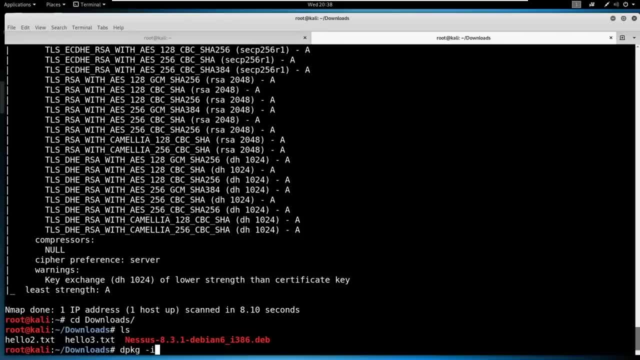 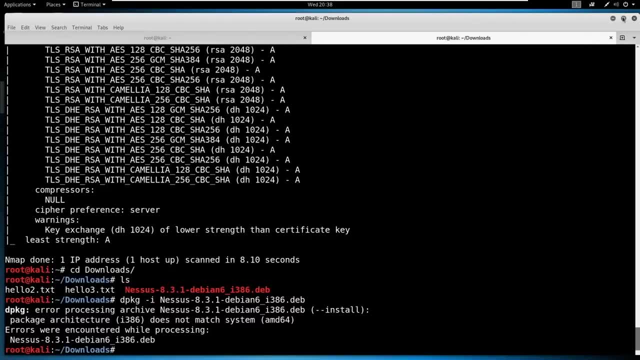 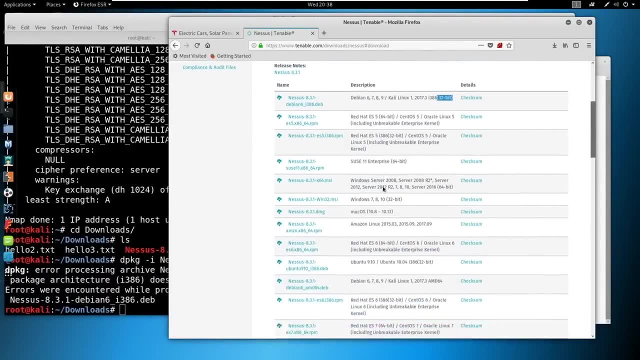 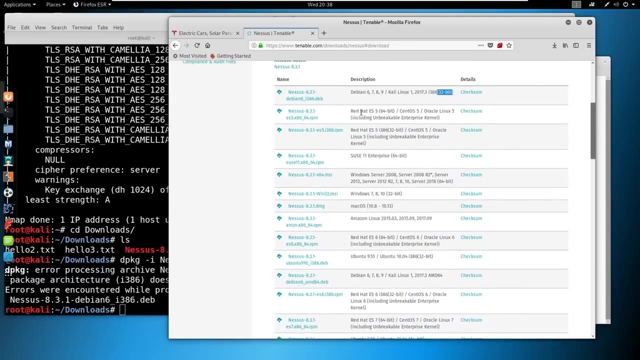 to do dpackage like this. dash i nessus and I downloaded the wrong one because I'm an idiot, so give me a second. I downloaded the 32-bit. don't be like me. there should be a 64-bit floating around somewhere. 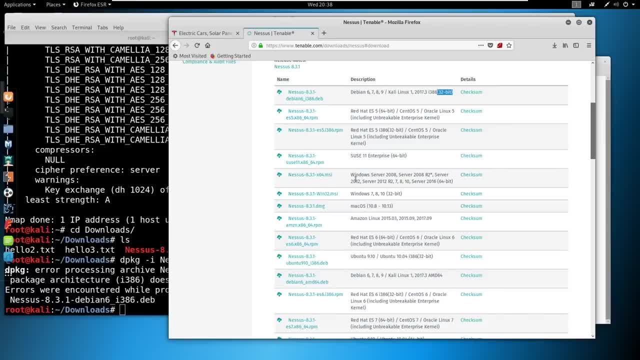 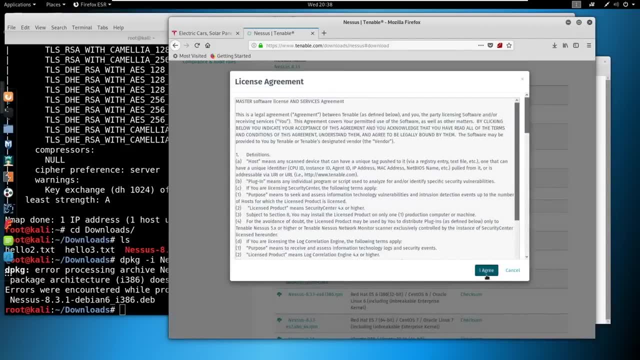 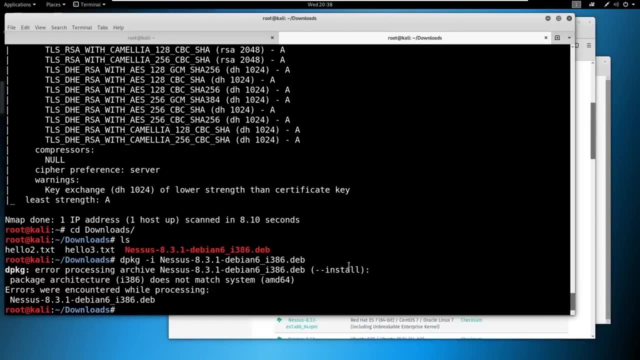 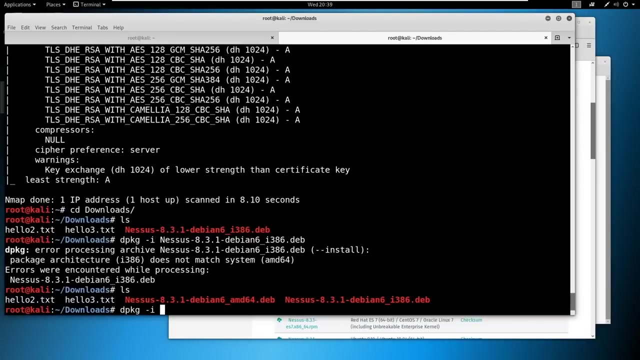 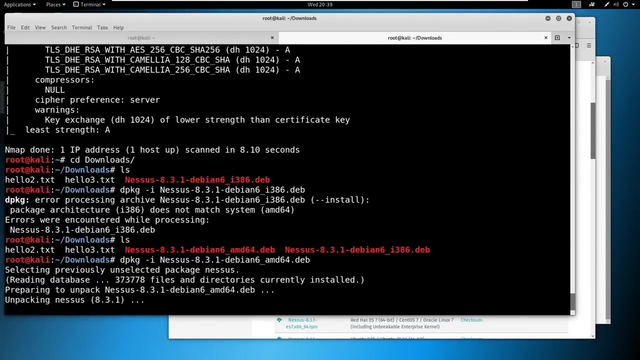 or I could be way off base here. There, it is a little bit down the page, guys. all right, let's try it again: dpackage dash i nessus, and we are using amd64.. Okay, there we go. 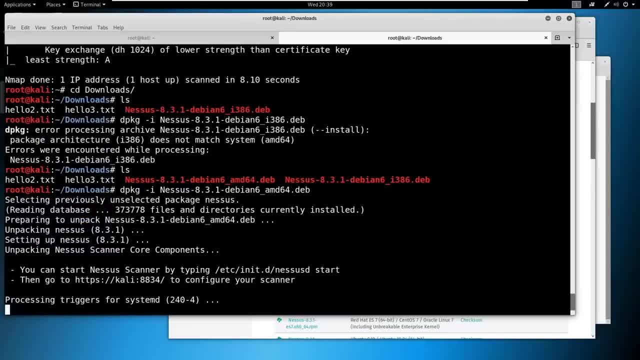 Okay, now this is installing. this will take just a second And it's done. All right, so you can see. it tells you to start your nessus scanner by typing in this: etsy, initd- nessusd- start. we covered what that does in week one, right? 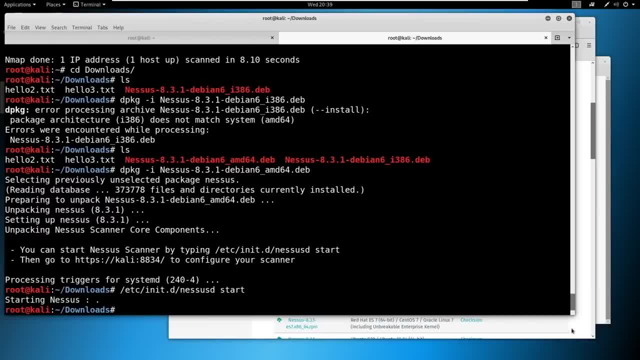 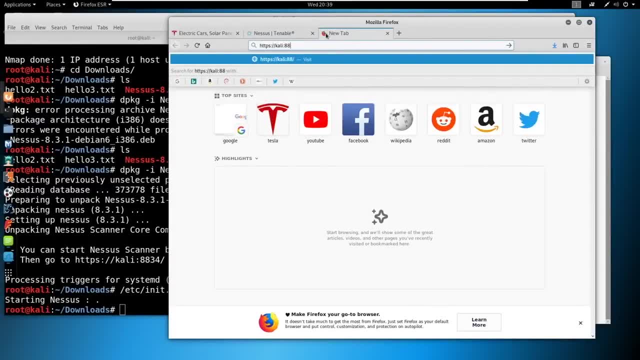 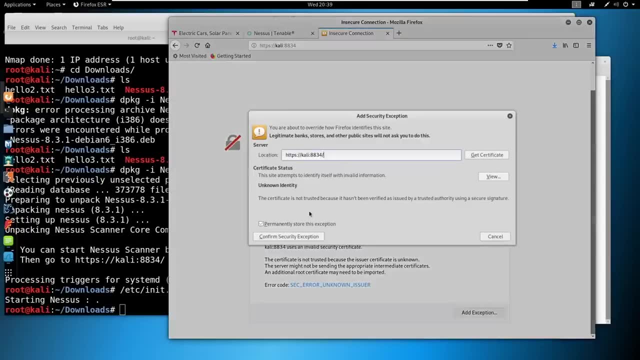 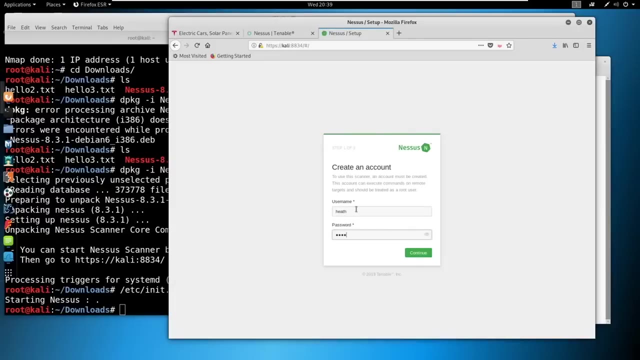 And now we're going to navigate out to HTTPS: cali 8834,. this is pretty default. You can also use your local host if you'd like. Add the exception. confirm the exception. all right, you can create an account now. 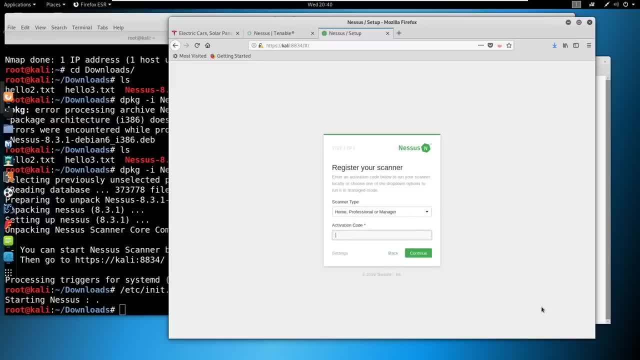 And we're installing the home professional or manager. we're going to use the activation code that we downloaded, And that's not it. Okay, I can't copy paste to this workstation. I forgot about that, So we're going to type it out the old-fashioned way. 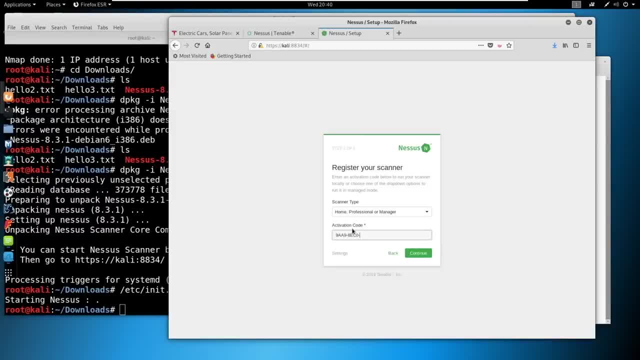 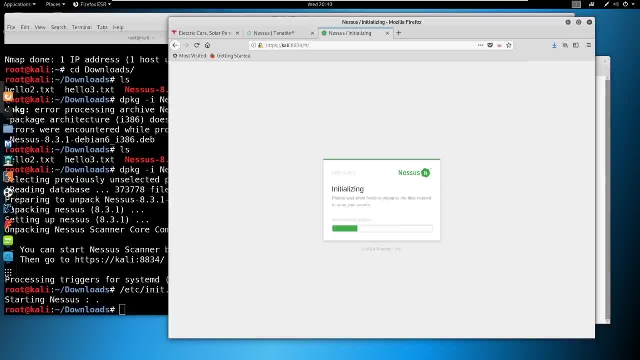 Yup, this is going to be a long part, So we're going to actually skip around, bounce around here for a minute while this is going. Print screen: You can have this one. this is the home version. Thanks for the sub Pong. I appreciate it. 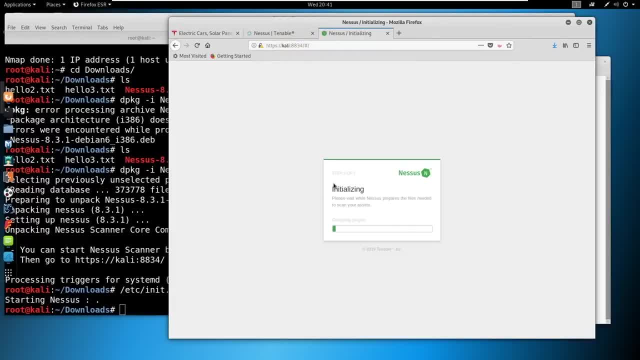 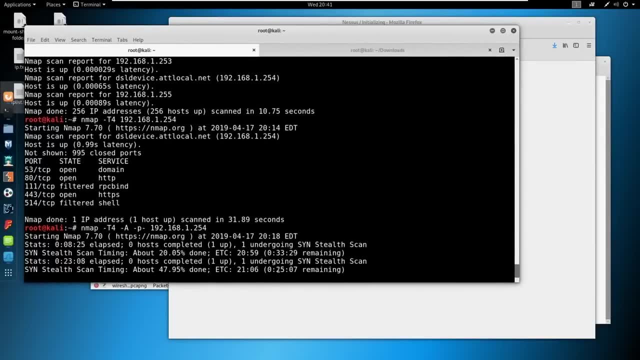 Okay, so this will take a minute, All right. All right, This is the home version. This is the Home version and let's check on our scan over here. we're still at 25 minutes and 17 minutes has gone by, but we've only lost eight minutes, which is not a good sign for us. 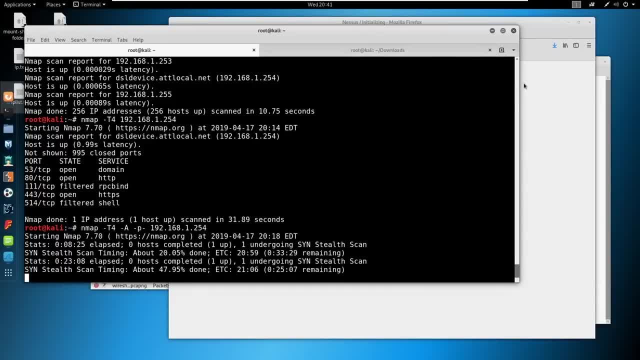 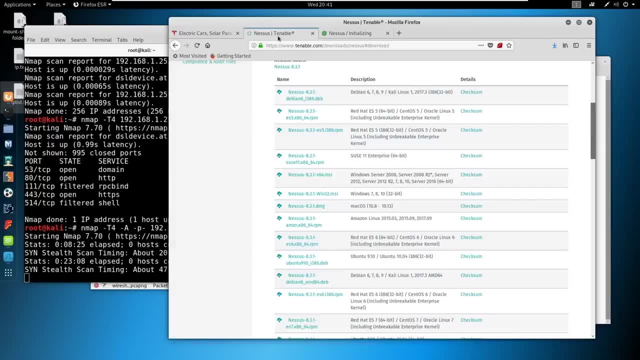 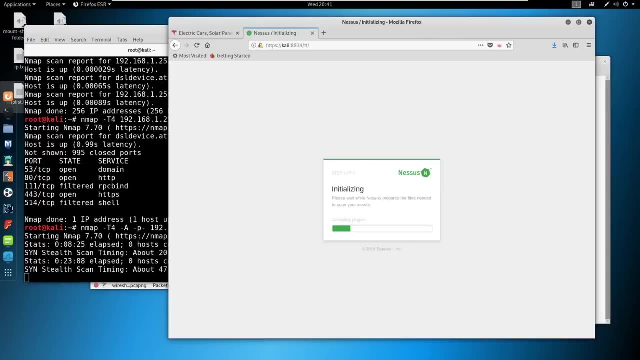 you want to hack Facebook, you need social engineering. for the most part, there's other methods. that would probably be your easiest route. all right, while we wait, we are going to look at Metasploit as a tool. it is a fantastic scanner of all sorts. we're going to be talking about using its port scan feature, which I don't really use. I'm just 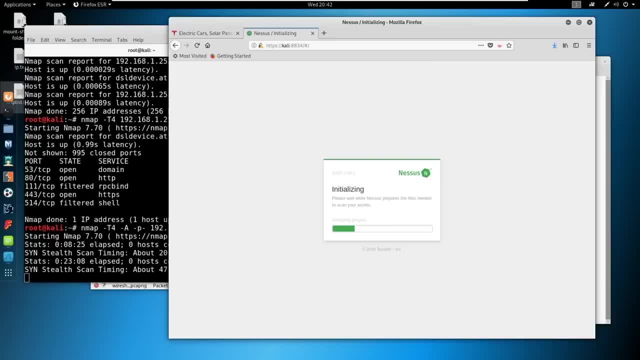 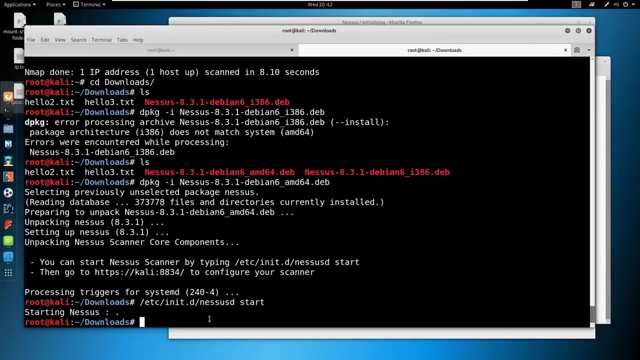 doing as a proof of concept, but we're going to talk more importantly about the auxiliary feature and the fact that there is a scanner in Metasploit. I will open this. Thank you for sharing that. I appreciate it. Okay, So in order to start up Metasploit, we're going to just type in MSF console. 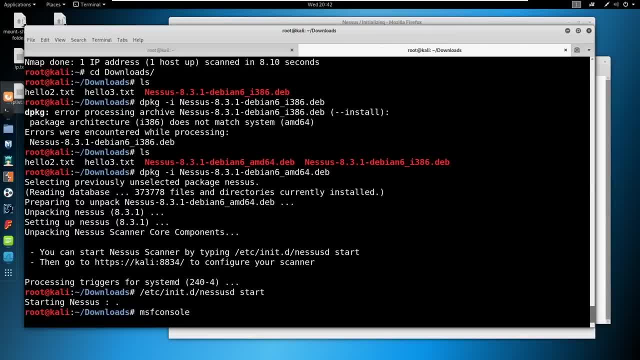 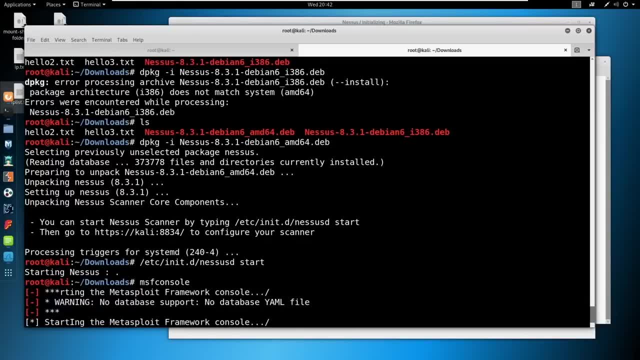 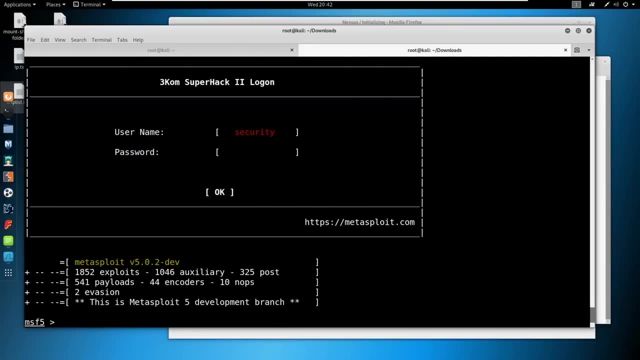 Not in all caps. that's bad. Um, this will also take a quick second to spin up. depending if it's your first time or not. I don't even know if this is our first time on this machine. It may be Okay. So there are quite a few different features for Metasploit. I think there's 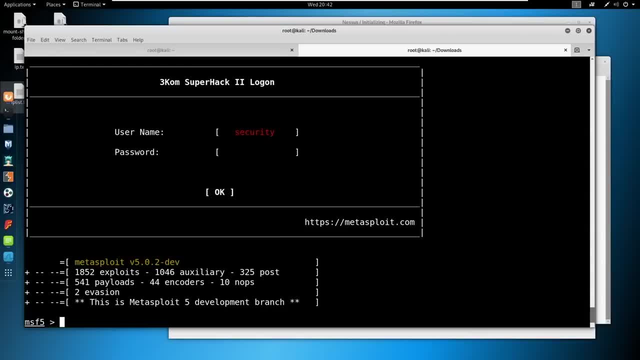 five different types of module types. I'm not sure how many module types there are. Um, the important ones to know is that there's the auxiliary, which is kind of like your beforehand, uh, like your enumeration, your scanning. There is the exploitation, which is 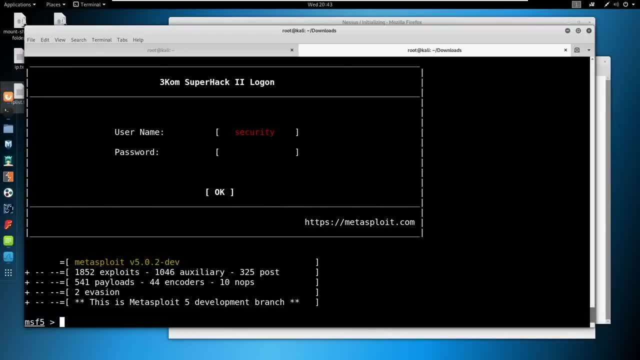 exactly what it sounds like. There are exploit modules and there's post-exploit, which are things you can do once you have a session. So we'll be covering all of these, if we need to, as we go through the course and, uh, you'll get it to work. 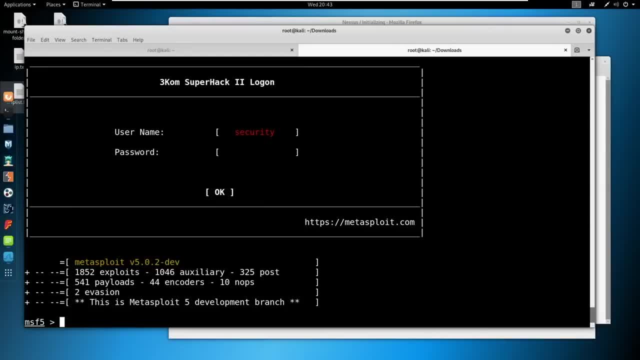 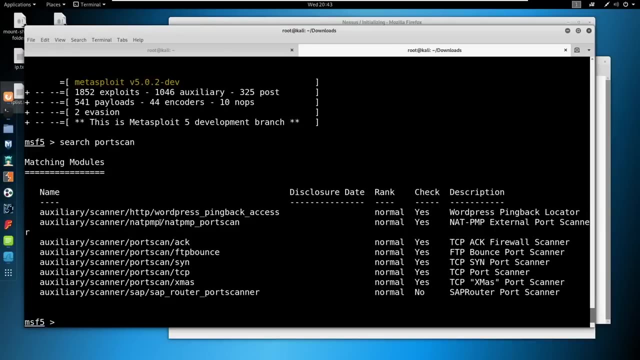 Okay, So now let's just go ahead and we're going to type in the word use. Actually, I'm going to show you a search. first We're going to search port scan And you can see there's a few different port scanners in here If you look at auxiliary scanner. 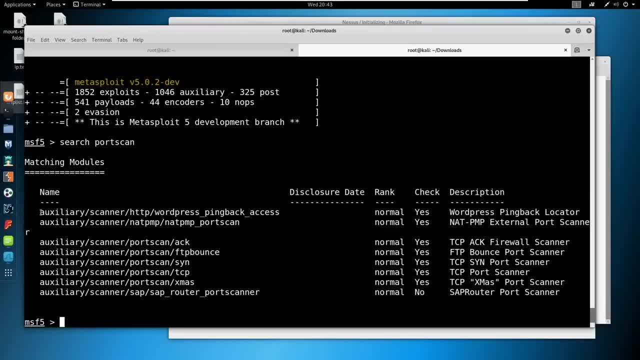 um, so it kind of goes by category, right. The first category is auxiliary, The second one is scanning, And then it tells you what it's going to do. Well, this is on HTTP and this is a WordPress pingback access. Uh, the one we're looking for is: we want to do a, a scan. right, We can either do. 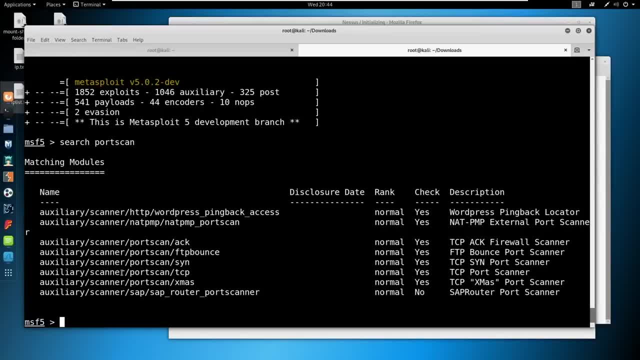 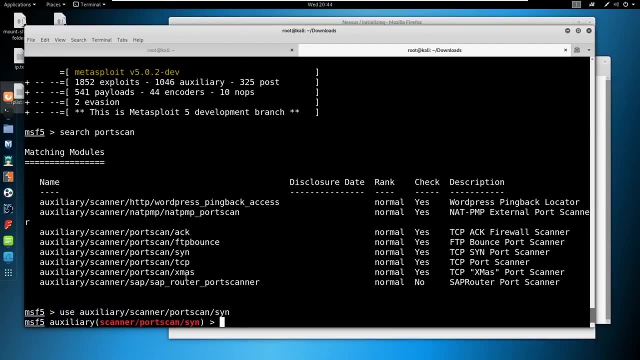 a TCP scan or a SYN scan. It's got a bunch of different ones here And we can just copy and paste this. So we're going to say use, we'll paste this in here. A couple of things we can do here If we want to find out what a module is all about When we go. 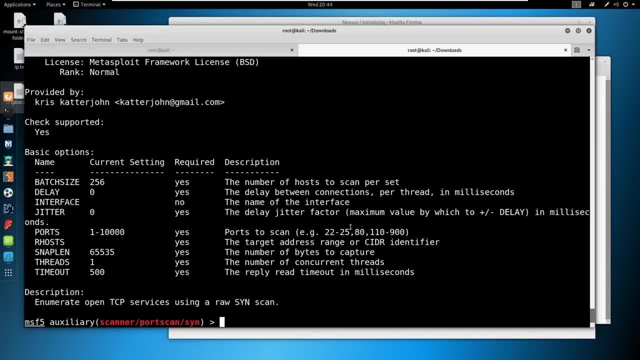 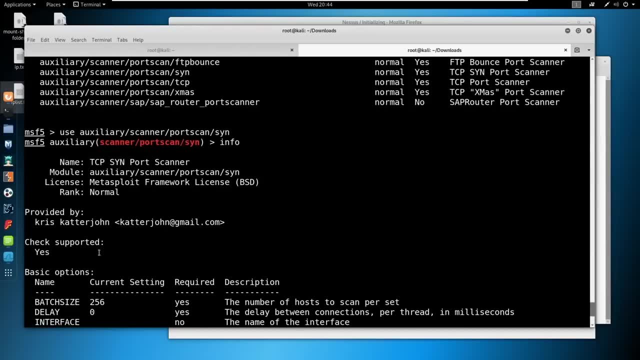 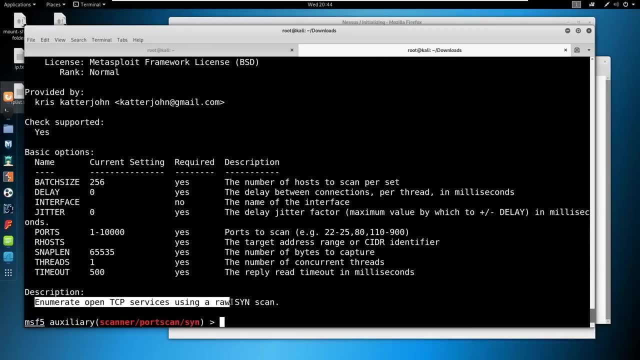 into it. we can say info gives us a little bit of information on it. So it says: the TCP SYN port scanner tells you who it was built by And it gives you some of the basic options. Description here is enumerate open TCP services using a raw SYN scan. 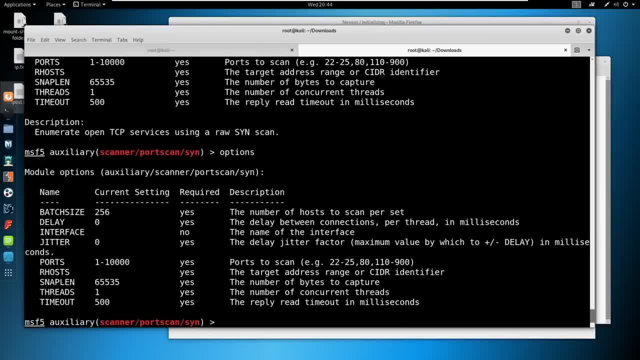 Okay, Now we can also just type in the word use. Type in options Doesn't give us the whole shebang on the description. If you already know what you're you need, then we just kind of want to see what options we have. It's important to 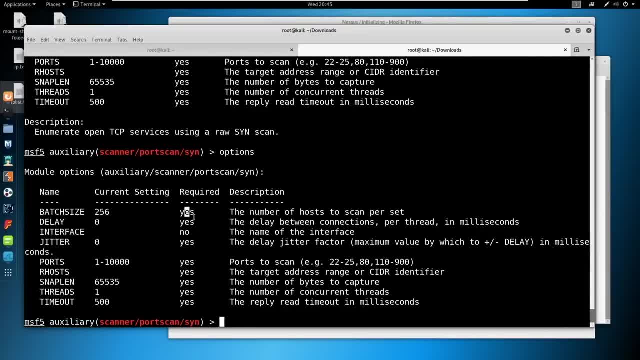 look through these and see what's already set and is required and what you still need to set. So if we look, this is scanning one through 1000 on ports. We might need to change that if we don't want to. It's scanning no our host right now. So 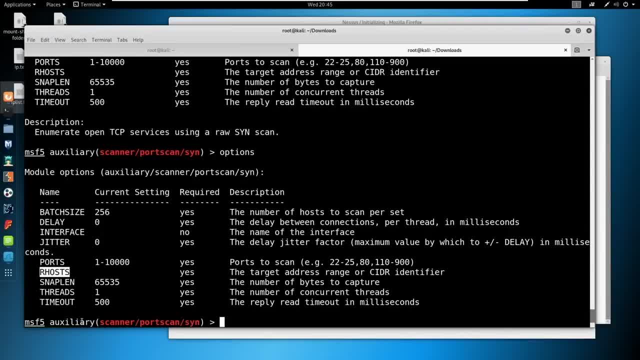 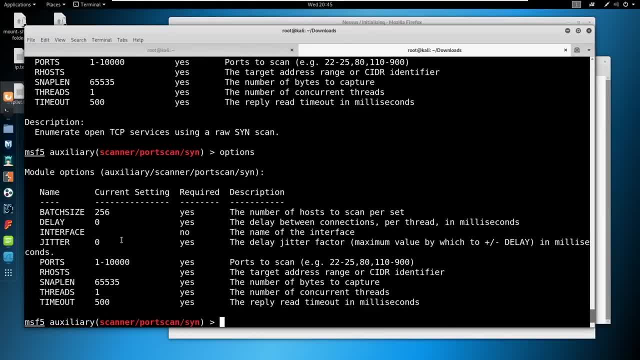 number of threading that we do here to increase the speed of these scans. we can. it looks like they've got delays, batch size et cetera. Importantly, what we're just going to be doing for basic syntax right now is we are going to say set and then ports, And I'm just going to change. 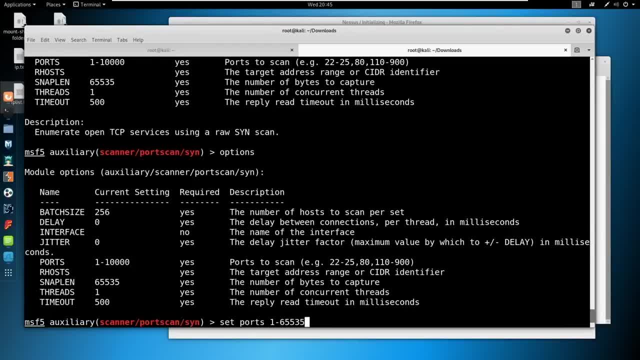 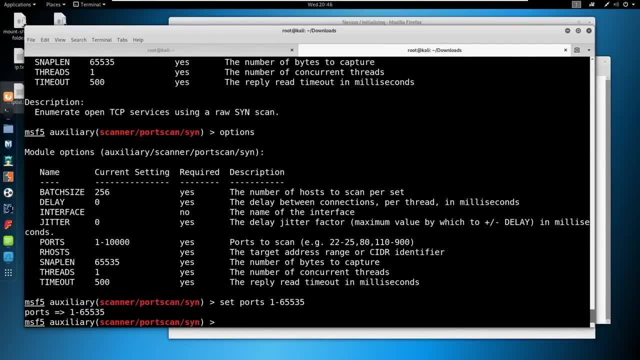 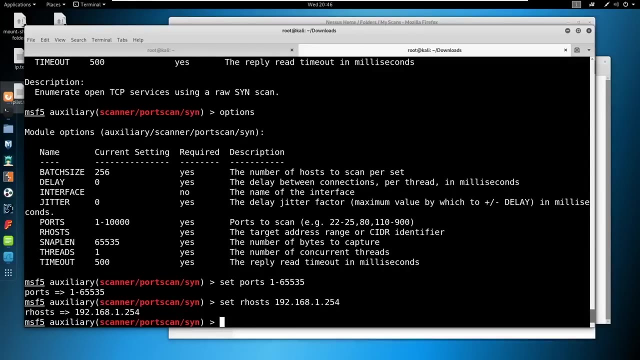 it to one, to 65, 535.. And then we're going to set in our host. So set our hosts, And we're just going to say 192.168.1.254.. So you'll notice as we go along that there's our host and there's our hosts. Our host is when you 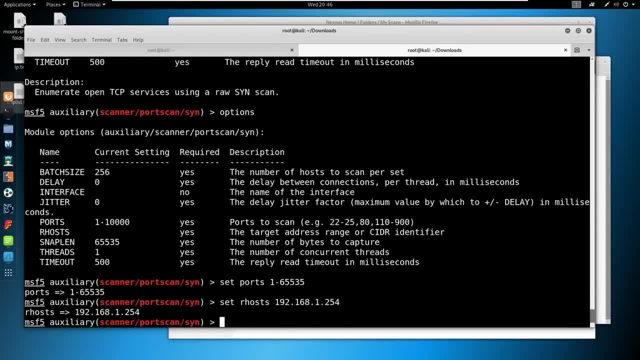 can only supply one address in the situation where you see an S on the end of it. you can apply multiple. you can apply a range Um some sort of cider identifier, as it says here. we were just going to be scanning one. 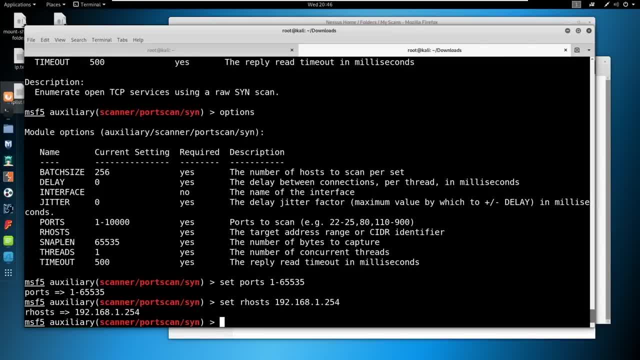 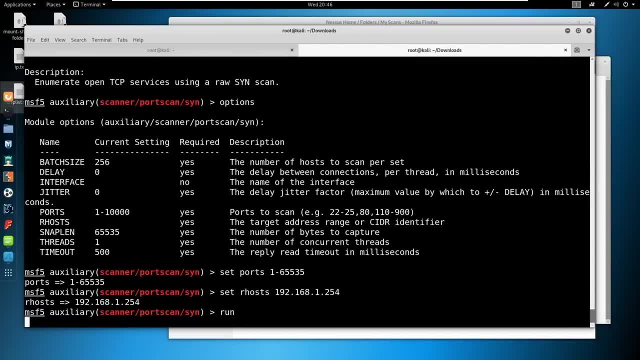 address, which is absolutely fine, And we can type in now run. or you can type in exploit, if you want to feel cool, And this will start scanning as well. Now, all this is going to do is tell you if a port is open or if a port is closed, And with all this traffic going to my 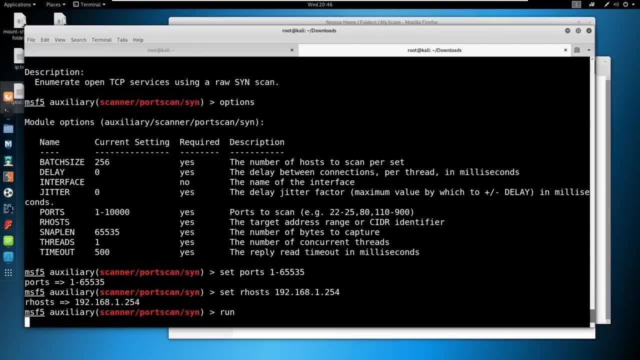 router if I deny myself service. it was nice knowing you guys. We'll see what my- my router can really hold up to. Okay, I'm actually going to kill this. Just want to show you proof of concept on how to run. 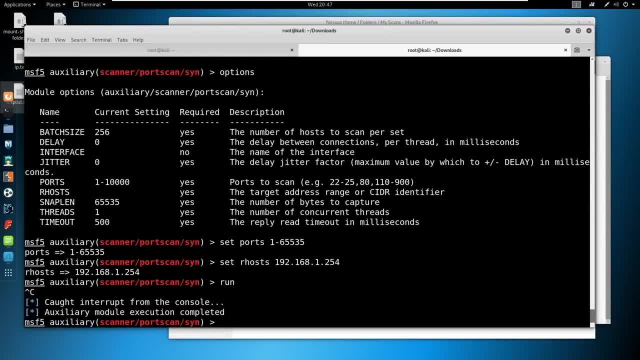 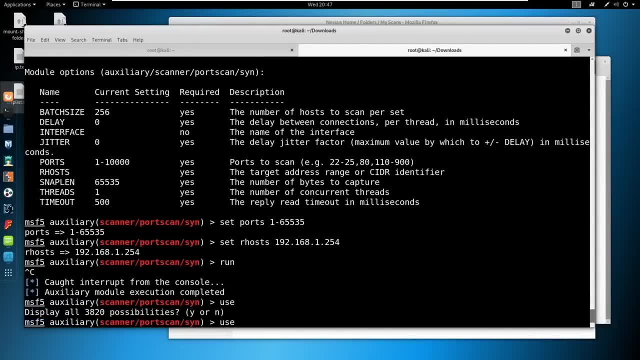 something in here. Most importantly, though, if we go back to use- let me just double tab- There's 3,800 possibilities. Uh, no, we won't do that. We'll do auxiliary, and then we'll double tab. There's still a thousand auxiliary. 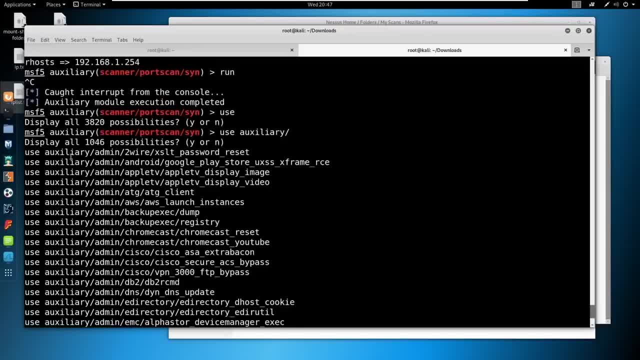 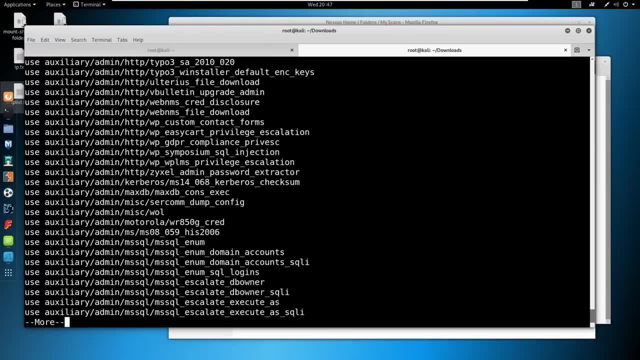 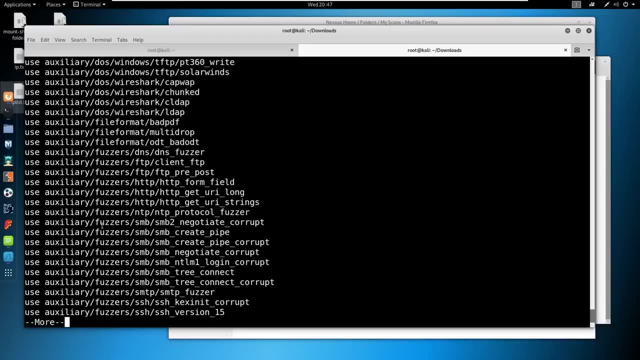 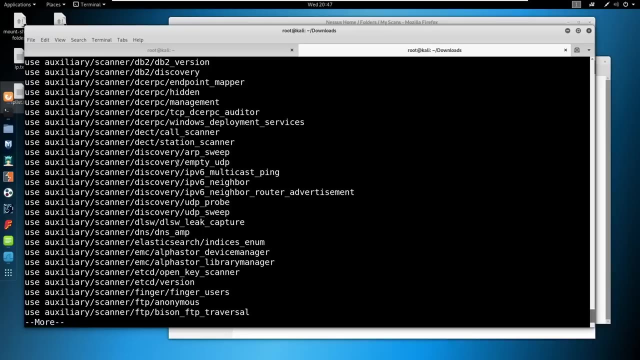 All right. So if you come through here, you can see all the different types of things that it does: Auxiliary admin: you just hit space. auxiliary denial of service windows, auxiliary fuzzing, gather, information gathering here, scanning all kinds of stuff. There is so much. 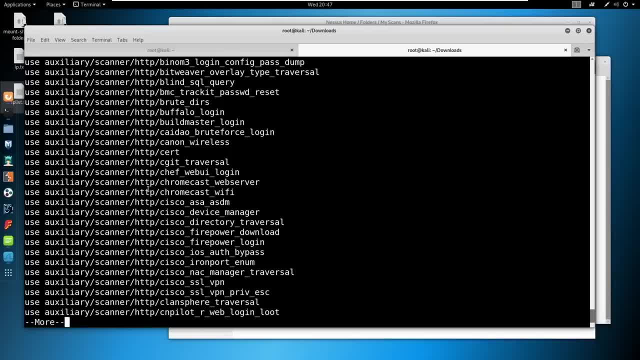 that Metasploit can do. It's amazing. So if you come through here, you can see all the different things that it does. Auxiliary admin: you just hit space, auxiliary denial of service windows- What you want to know- and hit queue. If you want to get out of this situation that you're in. 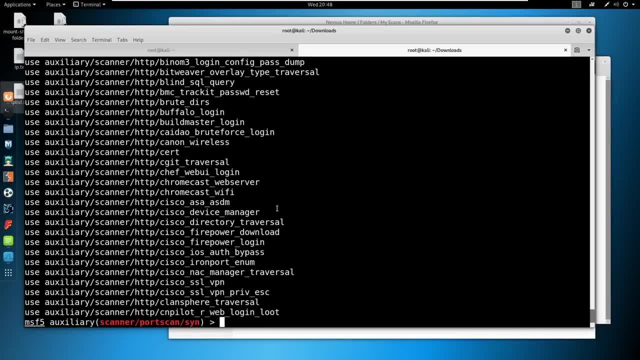 uh, what you want to know is what you're looking for. So say, for example, we found a Tomcat server and this really falls under enumeration that we're going to cover next week. But say: we found a Tomcat server and we're looking for exploits. You want to narrow it down to like search Tomcat. 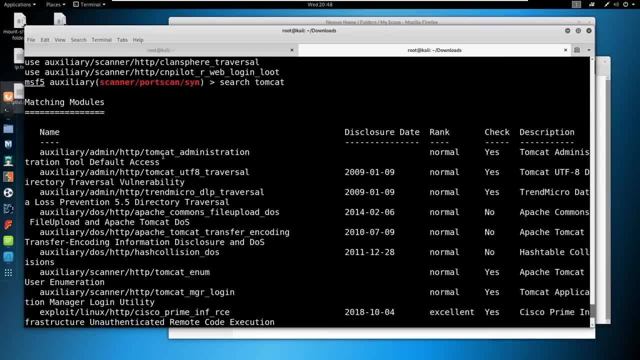 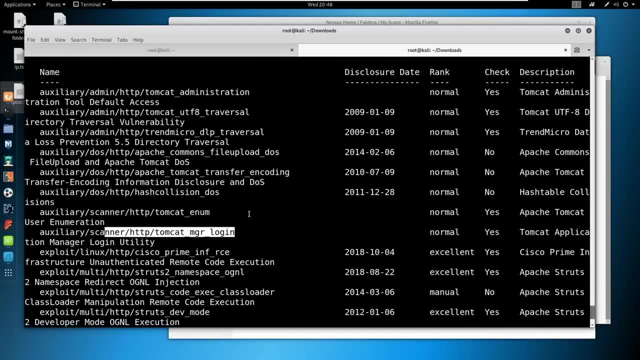 Okay, Then we can see what kind of things we have to maybe work with Um, Tomcat administration tool, default access. There's a directory traversal. Um. there's a denial of service. There's Tomcat and user enumeration. There's a manager login. There's. 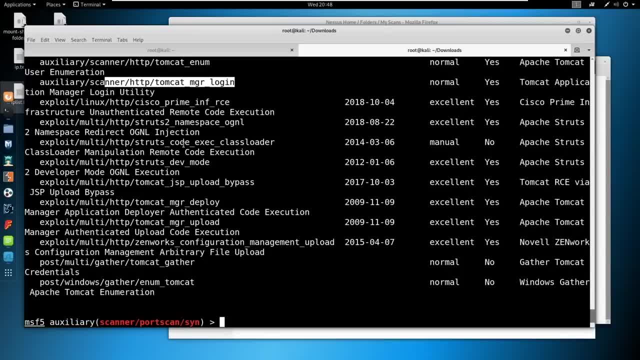 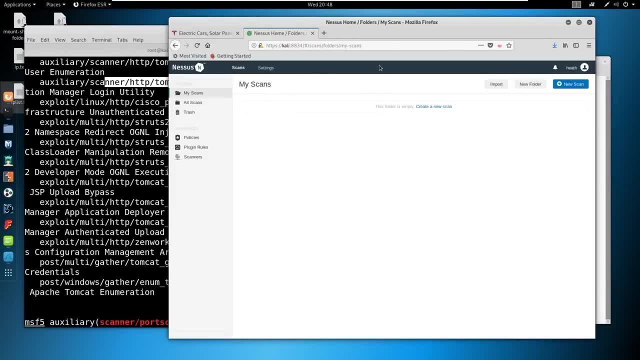 a bunch of stuff in here, So you might have to do some research as to what they are. And that's all part of the enumeration. So let's go back and check on our Nessus, see how far we are. Oh, we're logged in, Nice. Okay, So we get to scan up to 16 devices in our network. 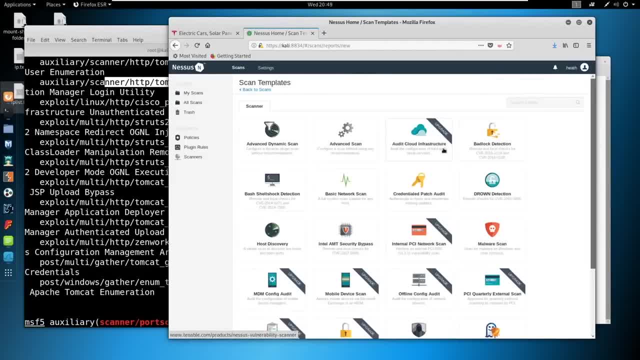 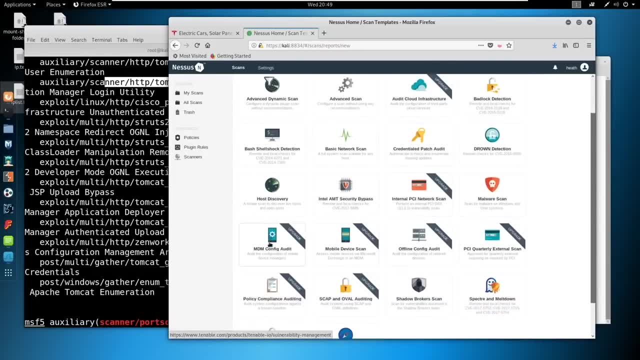 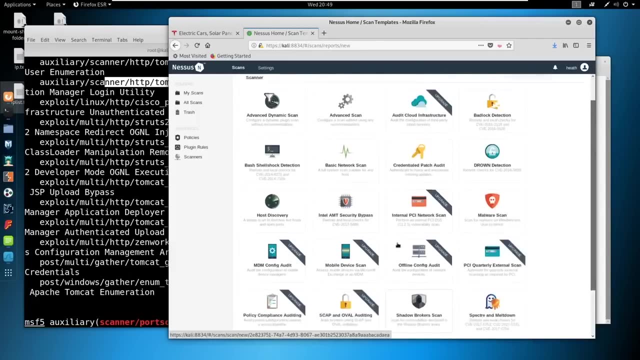 Perfect, We're only scanning one, At least I am. You can scan as many as you want. Now you can see what kind of um, what kind of things are prevented from being scanned here. A lot of this has to deal with compliance and auditing. Uh, so if you don't have the pro, 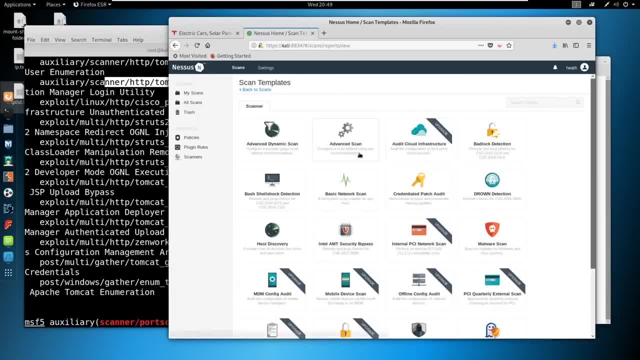 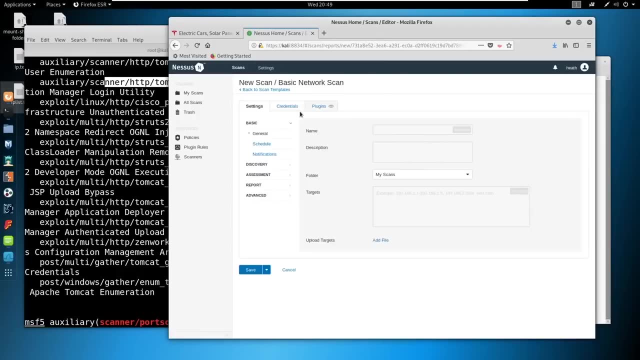 version. you don't get to do compliance and auditing. It's fine. Um, most of the time we can use this basic network scan. You can also dive around in the advanced scan if you want and see what that's like. Um, I used to use the advanced scan pretty heavily and now I've gone to just 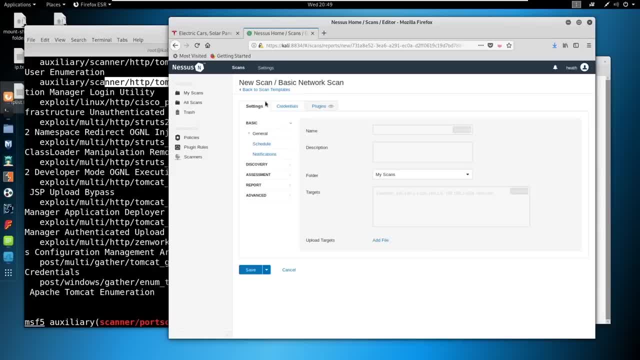 the basic scan, because I feel like it still catches everything that I need. Uh, so on this tab we've got our settings, which we're going to be setting here in a second. We've got credentials If we need to send um an authenticated session, say SSH or windows, and we want to scan internally. 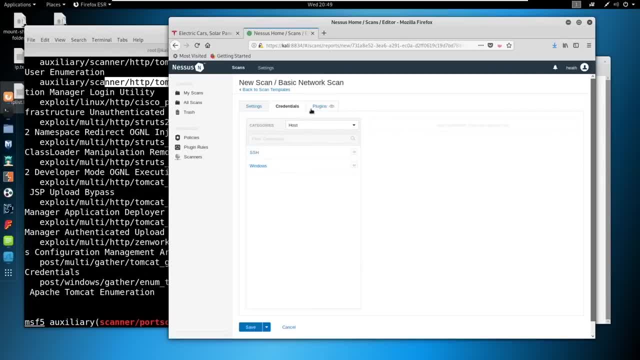 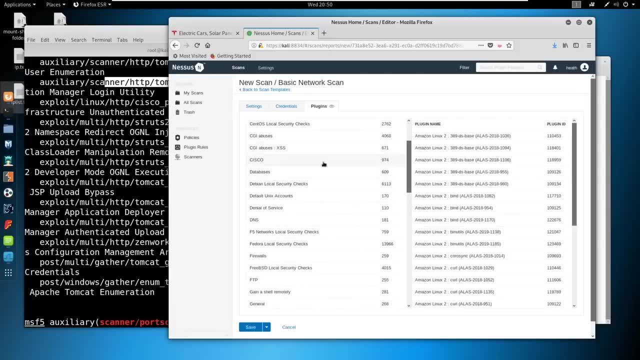 on a machine. we can supply credentials and get a little bit more information out of that machine. And then there's also different types of plugins that we have that we can run for. You can see all the different types of things it's looking for. Um, it tells you plugin information as you click. 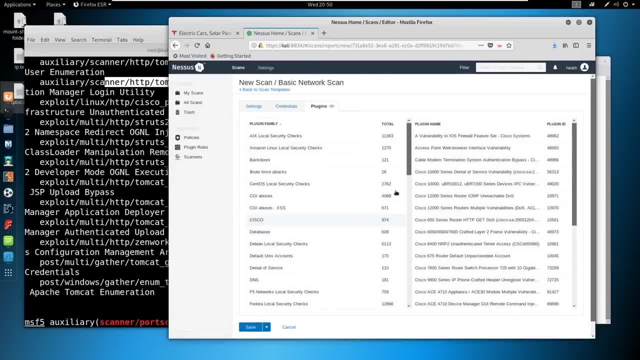 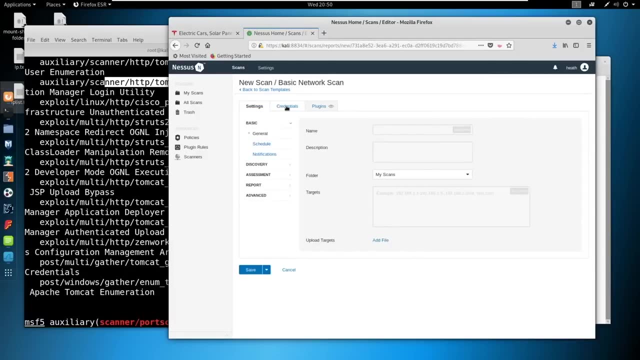 on it. So it's looking, for example, for Cisco. it's looking for a vulnerability in the iOS firewall. It tells you more information. So these are the plugins. It's best to keep your plugins up to date, if you can, so that you're scanning the latest and the greatest. So typically, when you're 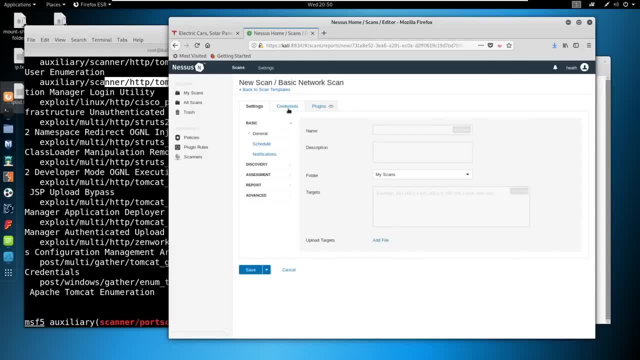 doing a penetration test and you're, you're scanning, at least on the external side, you're not going to be given credentials. Um, they're trying to make it as realistic as possible. Even if we're on the internal side, typically you're not given credentials. The only time we're ever really 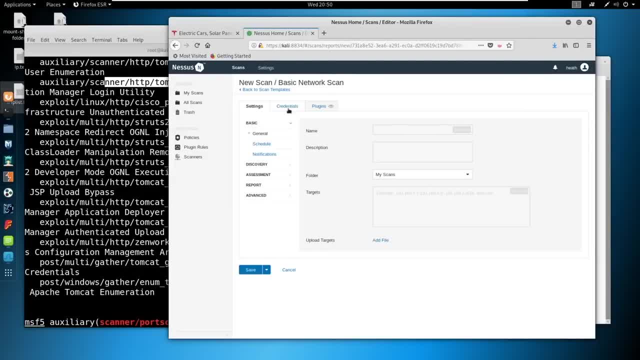 given credentials is for web apps, Um, and that's a whole different story and a whole different beast. So we have to earn our credentials and we're. typically this is more for like an auditing purpose, or I've used this in the past when I've been in another role to run an app scan fully onto. 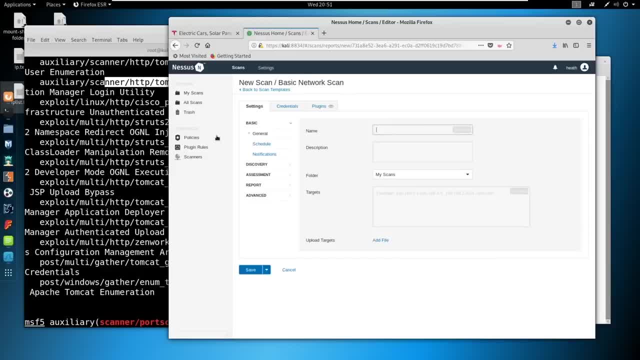 a system. So when we look at this, this basic scan, let's just give it a name. You can name it whatever you want. Uh, I'm going to name it my first scan, and I tend to just copy and paste that into the description as well. 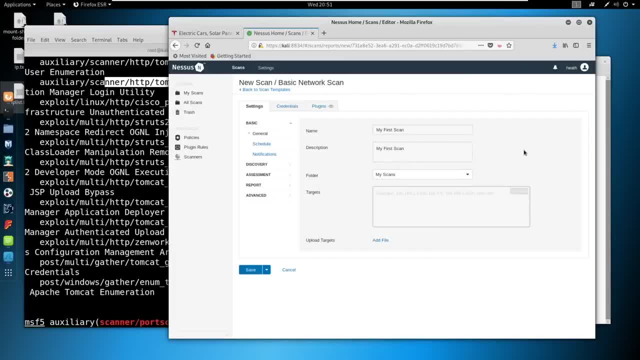 It gives you a folder you want to select. I just leave it as a default um my scans. And then, lastly, we need an IP address that we're going to be testing, Which for me is 1.254.. Now you can do all sorts of things. You can do 192.168.1.0, slash um, say 29 or or whatever here, And you can do like teslacom. You can set all sorts of different methods here, as long as you're separating by a comma. 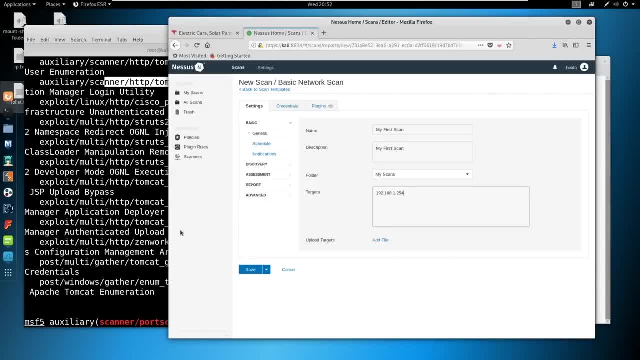 Okay, we can enable a schedule if we want. Um, this is a a trick if you want to get your scans going at 8 am. If you know, you can start your work at 8 am. Uh, a nice little trick is to have your scan email started or your pen test beginning email start. So typically we send out an email that says: hey, we're about to start a pen test. 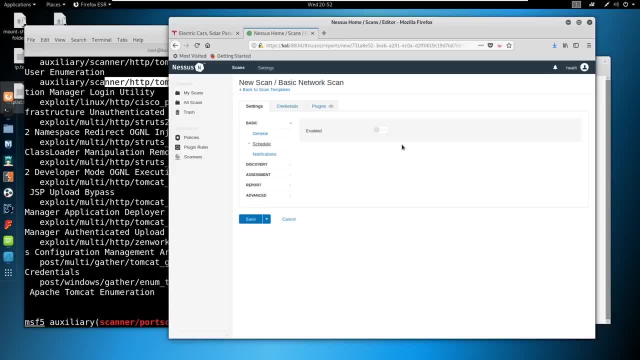 Okay, Just letting you know, Um, usually that goes out at the beginning of the day And at the end of the day it says: hey, we're, we're stopping pen testing for the day. Um, so you could schedule an email to send out at eight o'clock and you can also schedule your, your scan, to start at eight o'clock as well, so that they both start and you're doing, uh, doing a little bit of automated work. 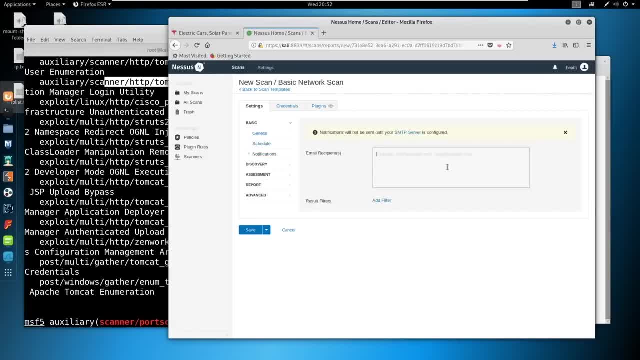 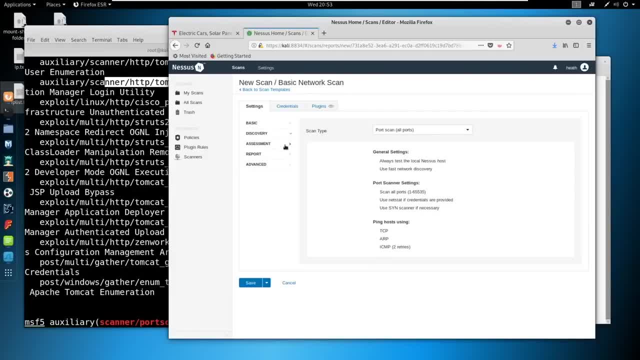 a. so we are allowed intentionally. That's almost the the whole part of being a penetration tester versus a red team. All right, We are intentionally loud. We want you to see our scanning activity, We want you to know we're there because we can help you tune your SIM- Uh, it can help get your blue team in line. And if you're not seeing this, these scans- what else are you missing, Right? So if you're not seeing the very loud scans, that's absolutely going to be a finding on a report. 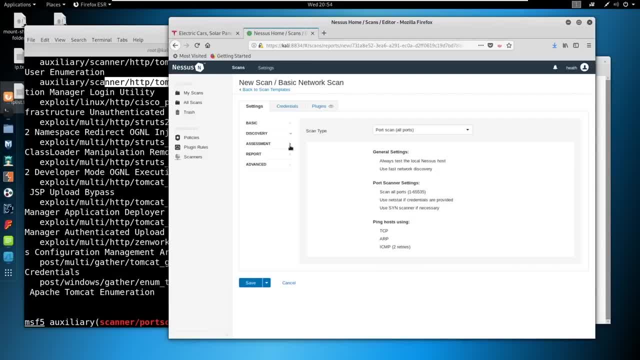 Um, so it's, it's important as a pen tester to try to be loud, to at least help the blue team, you know, catch some things and see what they're missing, what they're not. So we're going to go ahead and say port scan, all ports, And we come in here. Um, I typically leave this default. I have in the past scan for web vulnerabilities complex. but if you're doing a network external, that's really not important to um, even internal to be scanning for web vulnerabilities. 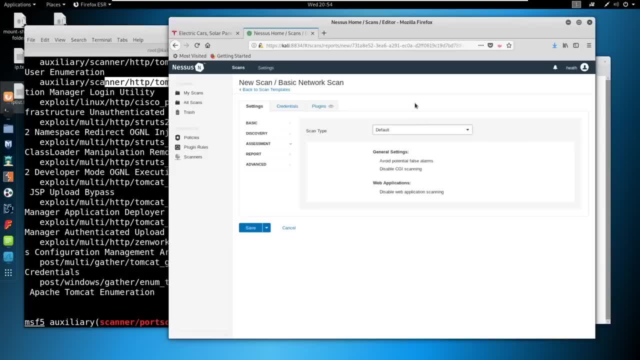 On the complex side, uh, unless you're doing a web app of some sort- So we've talked about this in previous streams, but I'll mention it here- when we're doing an external assessment and it has a website, um like, say, port 80 or port 443 is open, which is kind of common- Your, your job is not to be looking for issues with the website unless there's something that is particularly like out of place, Like if you're, if you get to the website. 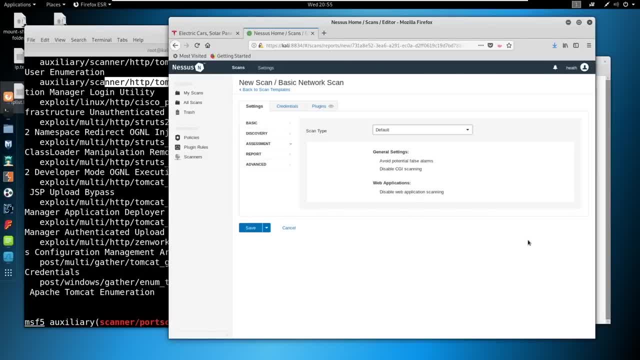 and it has a login screen, then maybe you'll try to do password spraying, like we talked about last week, Um, or you'll do credential stuffing, like we talked about last week, or you might try SQL injection, but you're not going to create an account and go in there and say, Hey, can I find cross site scripting? Um, you know what kind of headers are running on this server. Your, your job's not to do a web app assessment for that, or else they're going to um, pay for a web app assessment. right, There are two different things, Um. so what we're looking for is if 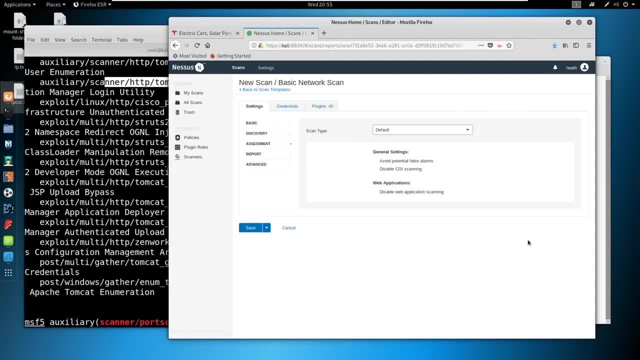 it provides some sort of easy access via the web. Okay, well, that's kind of in scope, Um, if you're you're sitting there looking for specific vulnerabilities on the website, that's really kind of out of scope, Um. so if we're doing network pen testing, which is what we're focusing on, we're going to leave the scan type set to default. You have a override, normal verbosity. This is all default. This is fine. The advanced side: let's see what's in here. 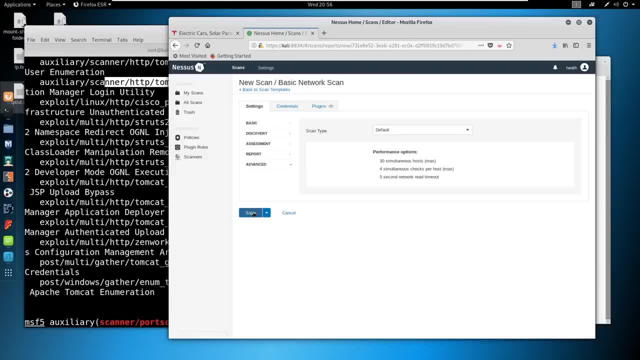 Scan low bandwidth links. I just leave this to default. Typically we hit save and then you come to this screen where it says my first scan. you hit this little launch button and launch off the scan. What can you do with your points? You want a t-shirt? Uh, I don't have any t-shirts, but we'll. we'll have a raffle here soon enough. I don't think you were around for the first raffle, were you? 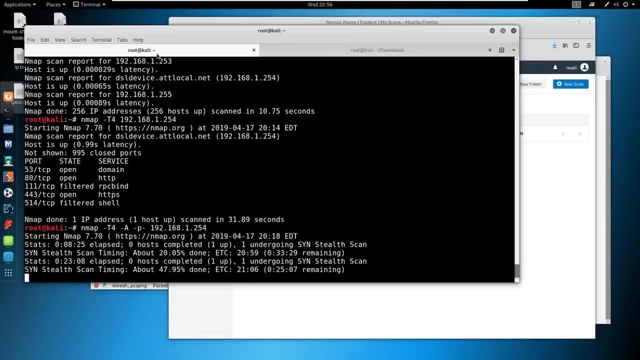 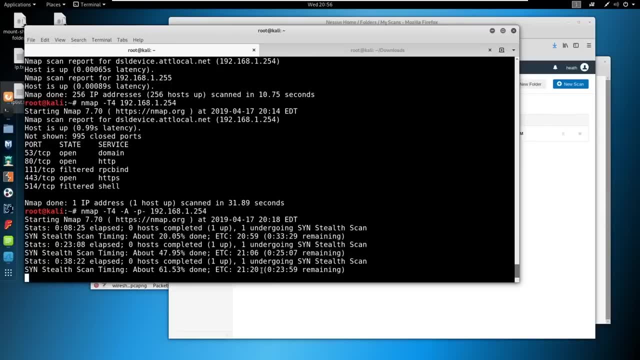 Let's check this guy while we're at it too. So another 15 minutes have passed and we've actually only gone down about a minute. So when I say network pen testing, would I consider that being called host system pen testing? Yeah, Host or system pen testing is another way to say it. 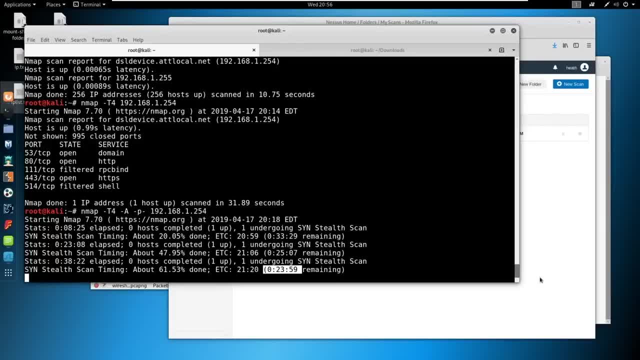 Donate for stickers. I do have stickers. I owe you a sticker Ion. but I emailed you. you never gave me your address, so you don't want a sticker that bad. Nobody wants my merchandise, All right, So with our Nessus scan. 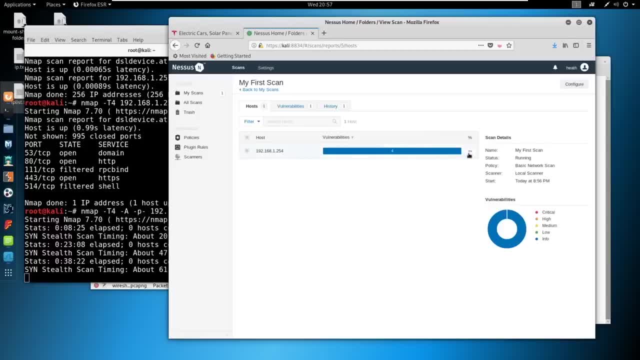 you can click in here and kind of watch it as it goes. You see we're at 0% right now And you look at the vulnerabilities, It's got a count of four. It's starting to find some stuff like it: found 53,, found 80, 443.. 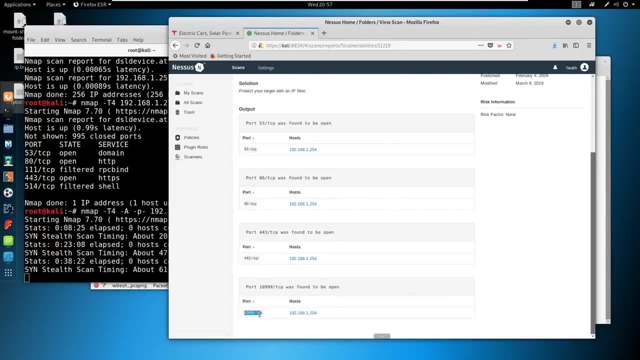 Ah, 10999.. It found an open port, So it's got. it's got some things here, right, And this is what. these are the kind of things that we miss when we just scan with the- the top 1000, right. 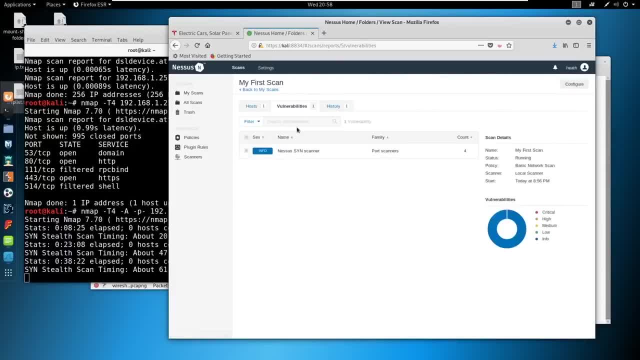 So critical to to scan everything you can. Now we're going to let this run. It's going to be a minute. It may even take the whole time. What we'll do, too, is if we run out of time or whatever it is. 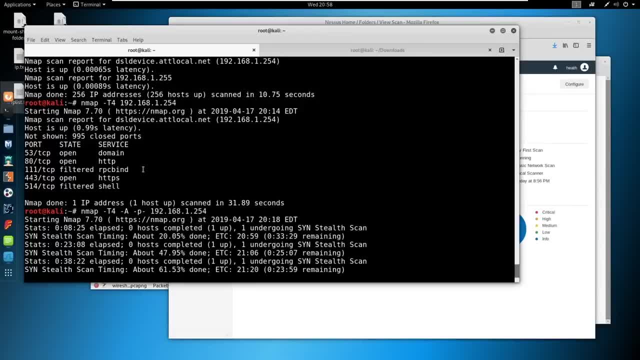 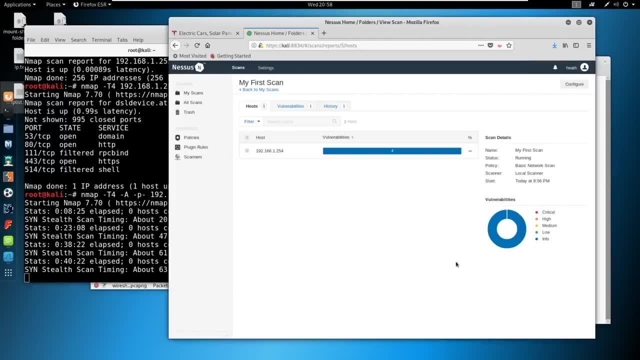 we'll go ahead and just check back in on the scans during the AMA and see if we can find any information, because this guy is running slow, All right. So while we wait on these two guys, we are going to do some web scanning. 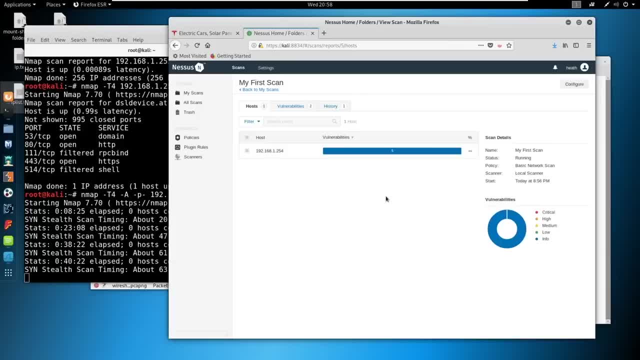 So there's two really popular web scanners: One is free, One is kind of free. So the popular is Nikto And that is built into everything with uh, with NMAP here. So it's built in, or not, NMAP. sorry, It's built into Kali and we're going to be running Nikto against Tesla. 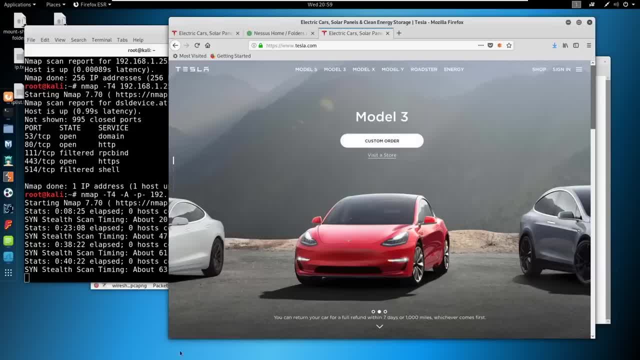 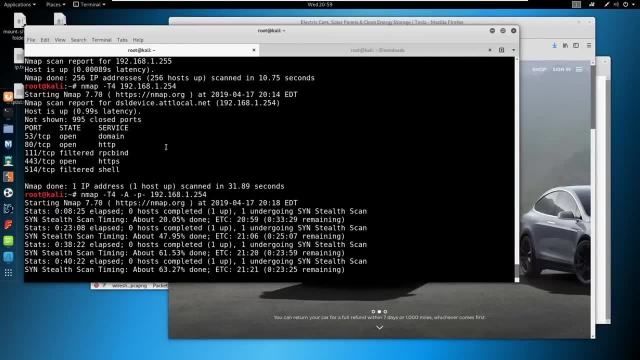 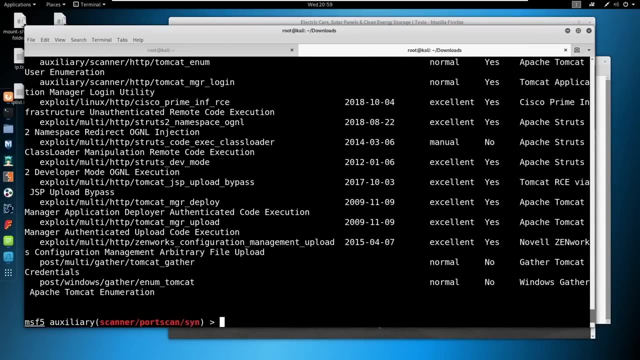 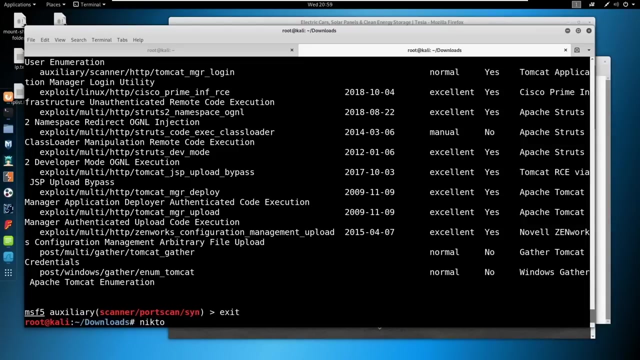 So go ahead and pull up Tesla If you want. you don't really have to. We're going to close, We're going to exit out of this And you can run Nikto from anywhere. Just type in Nikto And if we hit enter, it should give you some information. 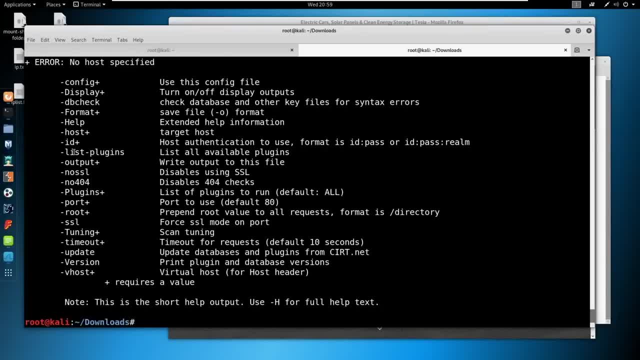 Okay, We didn't specify a host. That's fine, Let's see if we do a Nikto dash help like this: Same same stuff. Uh, unknown feature, A dash H is for a host, So we've got to supply a host. 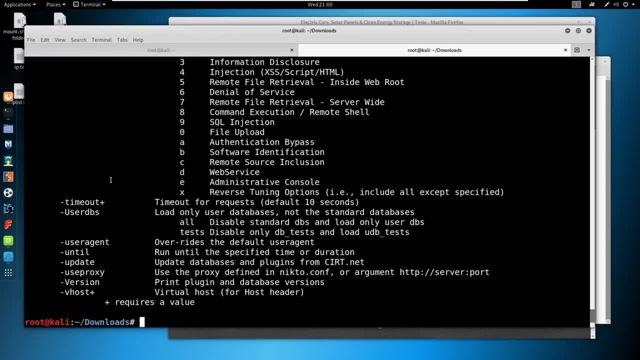 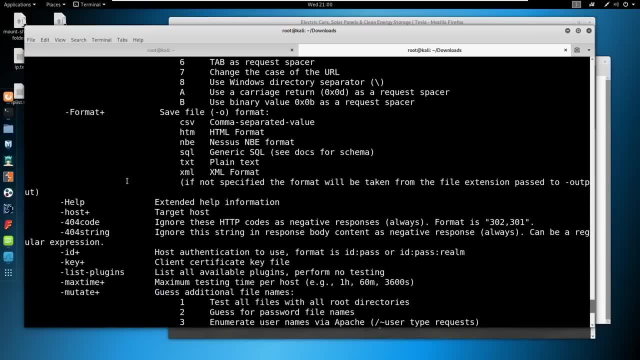 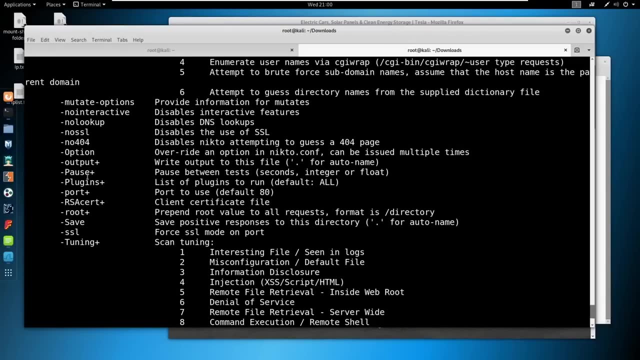 Ah, capital H. Learn to read. There you go. I knew that didn't look right, So there's quite a bit of features in here. Typically, we're going to be running this just as uh as is, But do know that there's quite a bit of things that we're going to be running. 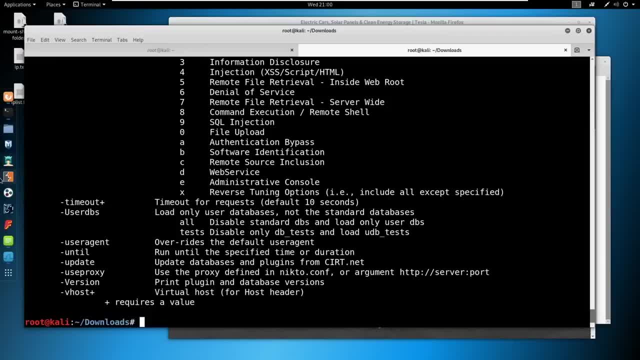 There's quite a bit of things that we're going to be running. There's quite a bit of things in here that you can do if you wanted to get advanced. So I want to run a scan against Tesla. I'm going to say: Nikto, dash H for a host. 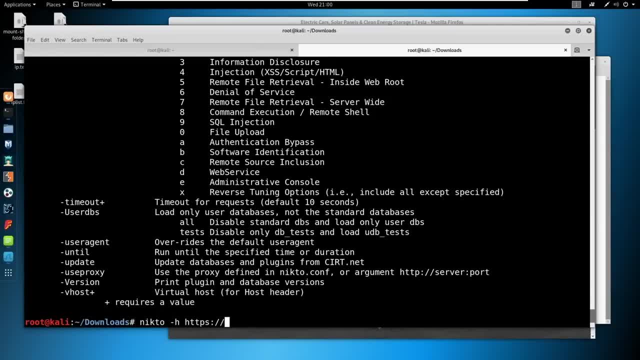 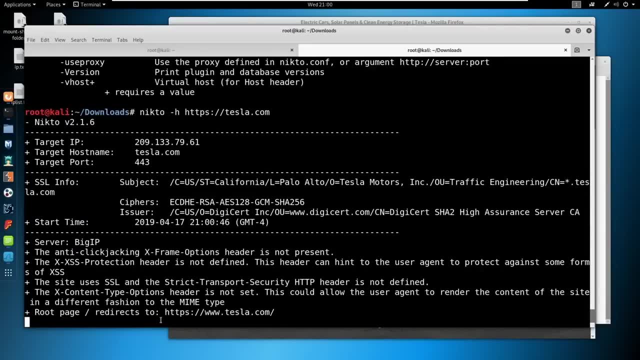 And then we're just going to say HTTPS. Unless it's HTTP, then we'll run it against that. We'll just say Teslacom And it'll start pulling information out At the end of the stream. can I post a summary of what we did? 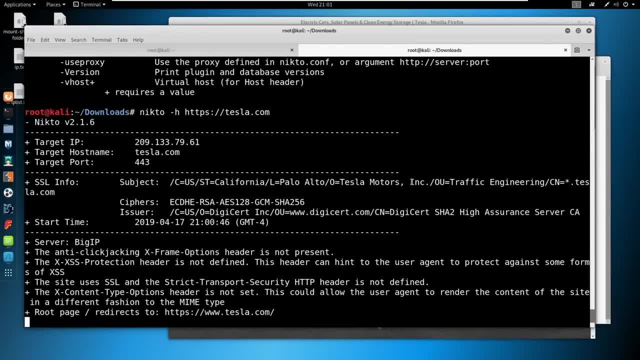 Um, I do upload these videos. You have the option to watch it on Twitch or watch it on YouTube if you'd like. Uh, so either of those would work out. if you wanted to recap what we did, I do try to timestamp on YouTube the best that I can. 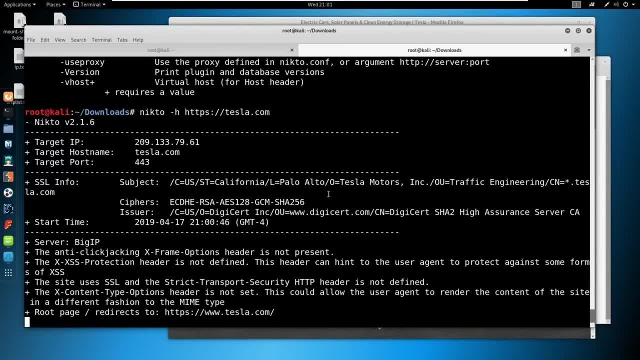 I don't timestamp the AMA just because we go through so many questions. but All right, So we come in here and this is basically just going to run a scan against all of this. So you see what it does for us. It pulls out an IP address of 209.133.79.61.. 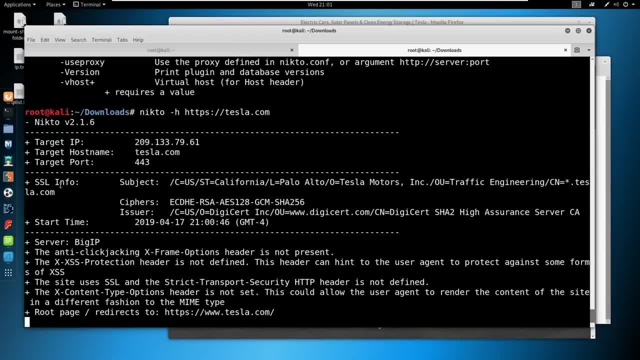 It's Teslacom, port 443.. It gives us the SSL info, It gives us their certificate, who. the issue is what kind of ciphers they're using. So a lot of information there, And then it's going to give us some more information. 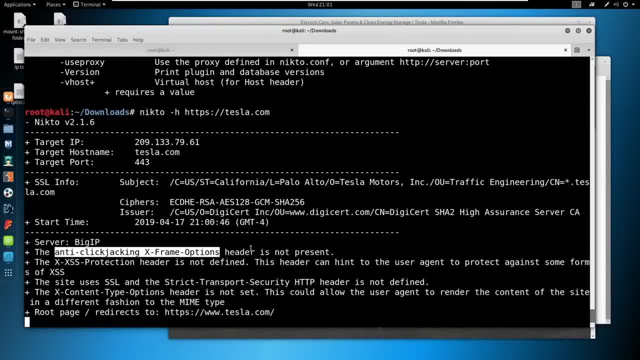 Uh, so So it says the anti click jacking X frame options header isn't present. if we're doing a web app, that's a like a low finding. uh, same with the cross site scripting header. That's a low finding. uh, there's no strict transport security. 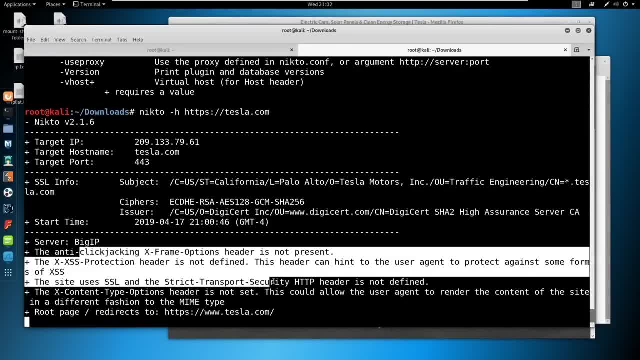 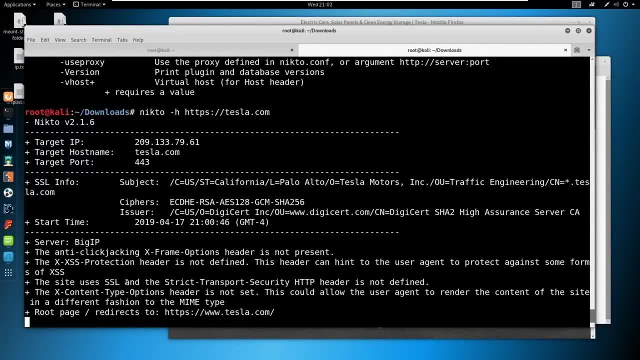 These are all probably be on one, finding um, just that their headers are not set X content type. Same thing. So it just checks all the headers and then now this is going to go through and it's going to look for um, it's going to do some, some vulnerability scanning. 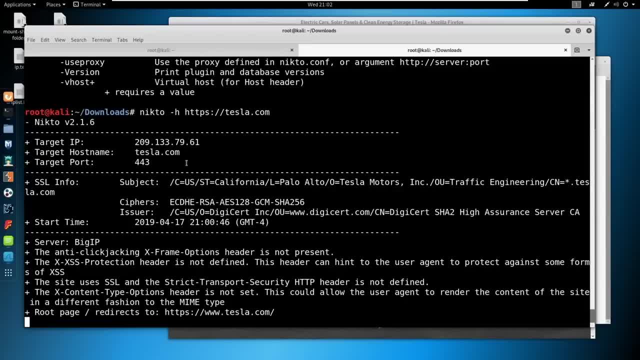 It's going to see If it can pull any sort of information based on what's running um on the web. And then it's going to say, Hey, you should look into this, this, this and this to see if you can exploit it. 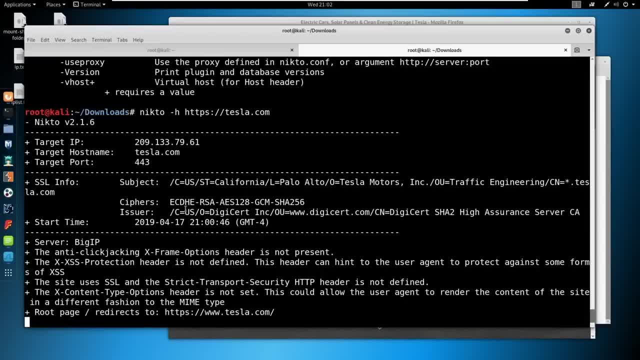 It'll do um, it'll do scanning and try to offer some suggestions on what might be exploitable. If it sees any type of um, you know, outdated frameworks or tools being run, then it'll it'll kind of look into this. 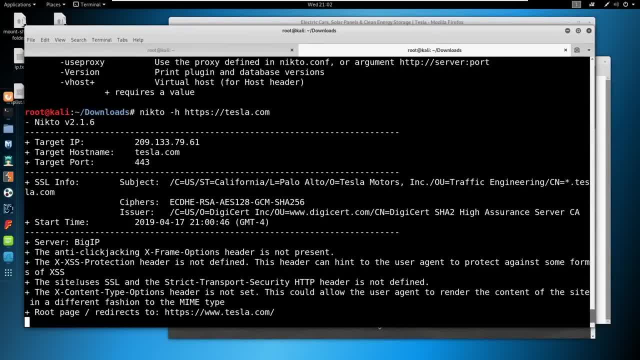 So we'll let that run as well And we're going to dive into burp suite. So I'm going to show you. I'm going to show you burp suite on here, and then I'm going to show you burp suite via my pen testing laptop or VM, I should say. 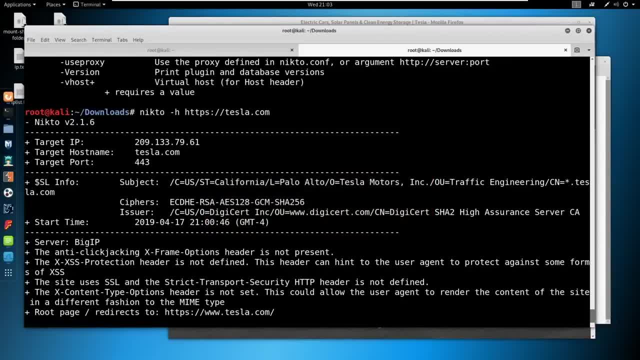 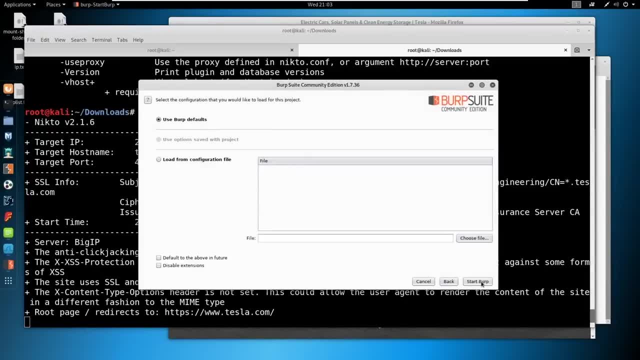 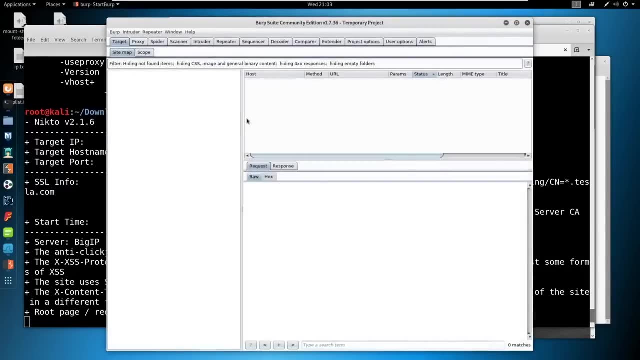 So this is burp suite community edition, and I haven't even set it up. So, uh, let's see if it works. Oh, this is 1.7.. Nice, This is. This is old. They're on the two edition now. 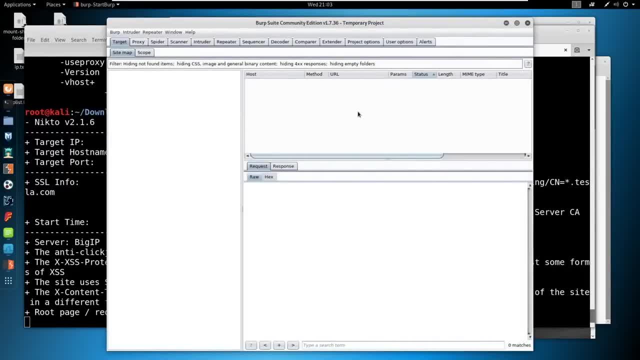 So you're going to see that mine looks just a little bit different. This is the most important tool that you can own, If you can invest $400 and you want to, if you want to do web apps and you want to do web apps right. 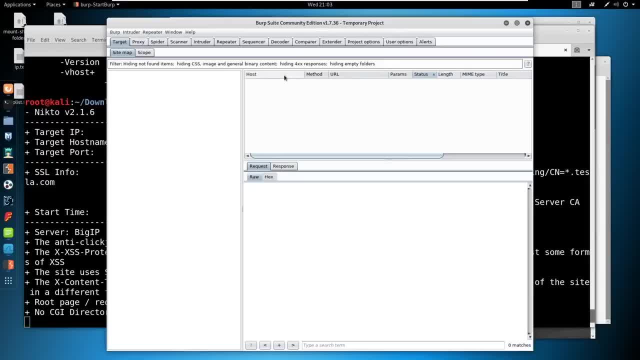 You need to invest the $400 to get the pro edition. Um, it has most of the tools in here and we're not going to be covering 90% of what they're doing. This this does because we're not doing a web app lesson right. 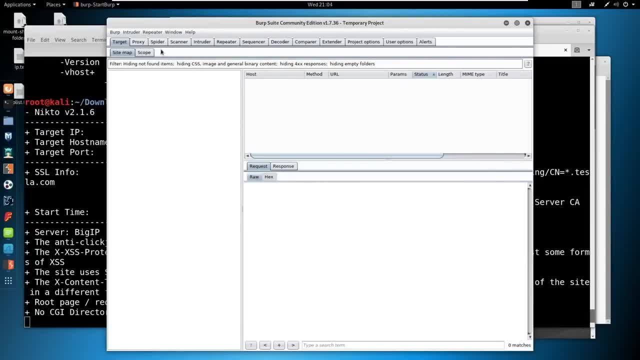 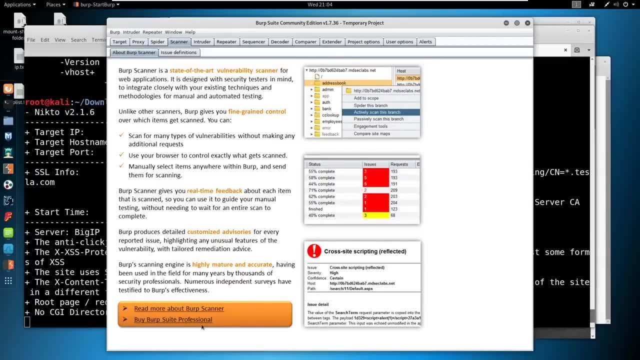 Um, but burp suite pro has an active scanner. So if you come into the scanner here, you can see that, uh, you need burp suite professional to do it. It is the one of the most important tools that you can own. 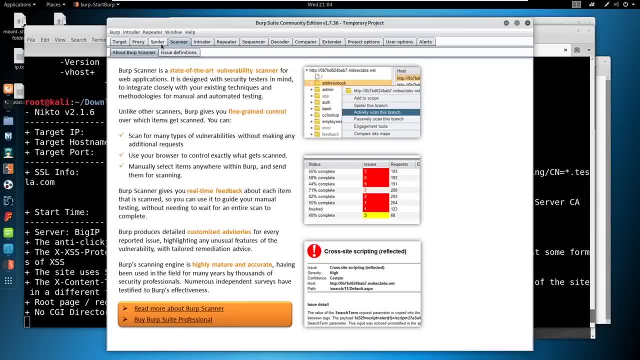 That's on the professional side, Um the that. and if you're, if you're starting a pen test company and you need to purchase two things and two things only, it's necessary, And it's burp suite, and that'll set you back maybe $2,500 to start your company, maybe three grand. 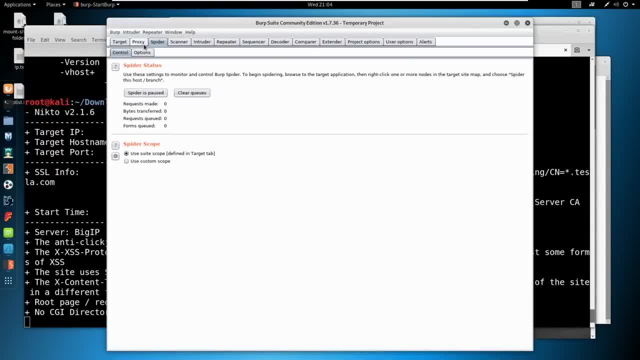 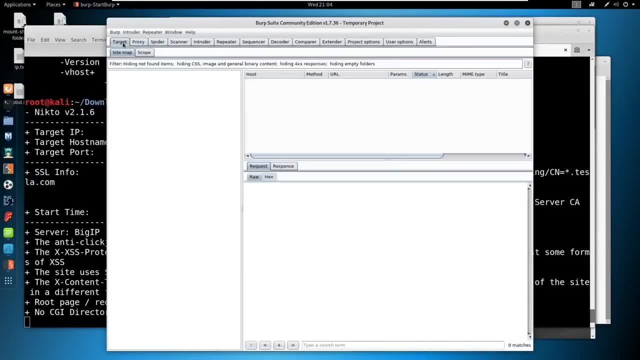 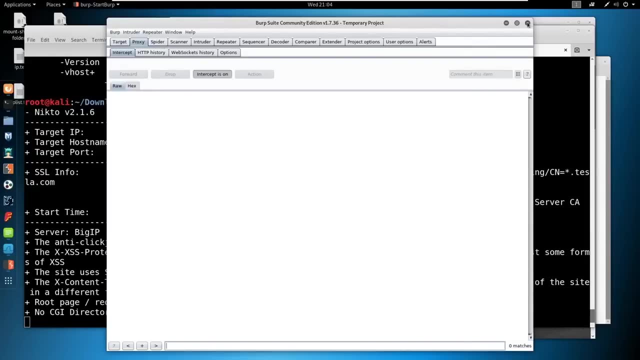 So it is a yearly fee. Everybody wants their licensing, Okay. So this is kind of what it looks like. I'm going to introduce you to the pro version so we can actually talk about scanning. Hey, I paid $400 for burp this year. 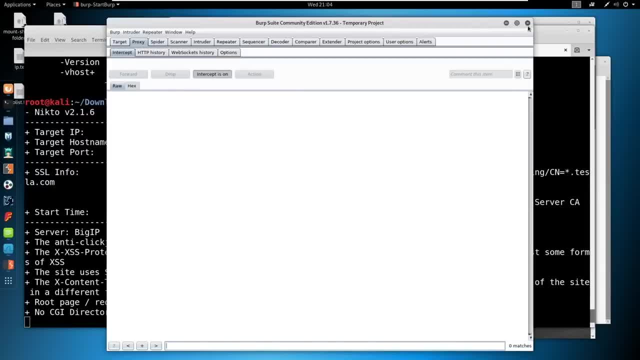 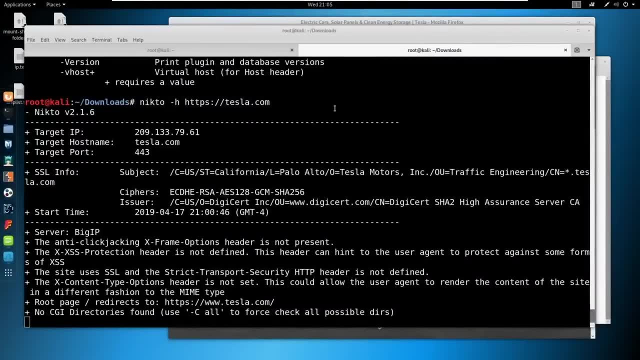 It was three, 50 last year. 2,500 for Nessa sounds about right. I don't know if they have a student discount or not. Yeah, I went up again. Cobalt strike is seven K. we have cobalt. I didn't I have no idea how much it is, but you don't need cobalt strike to do pen testing. 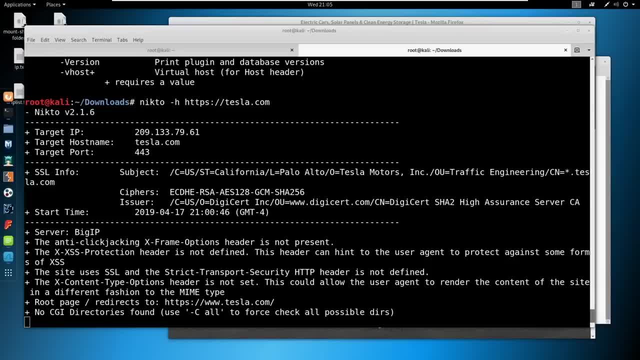 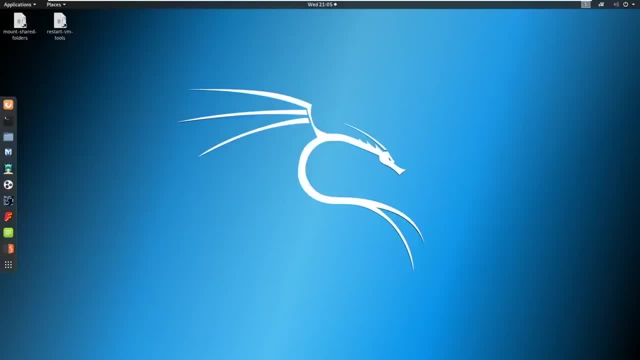 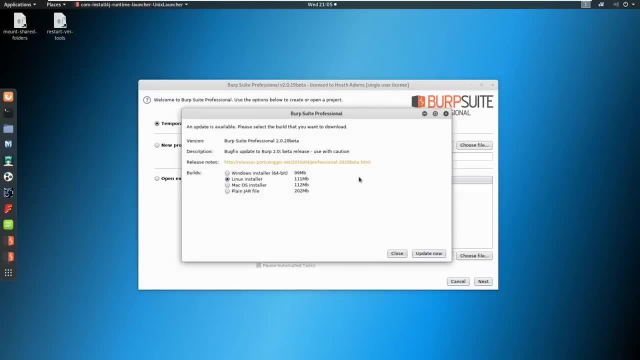 It's nice, but you don't need it. Um, here we go, Put this bad boy up. Hmm, This does wonders for you too, If you're doing hack the box or anything else along those lines. um, you can't use burp sweep pro on the OSCP if you're doing that, so you can use it in the labs. 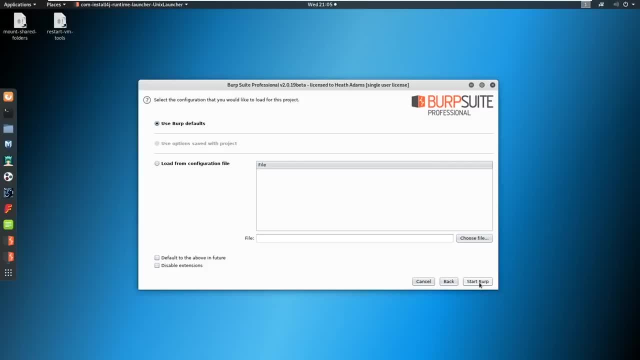 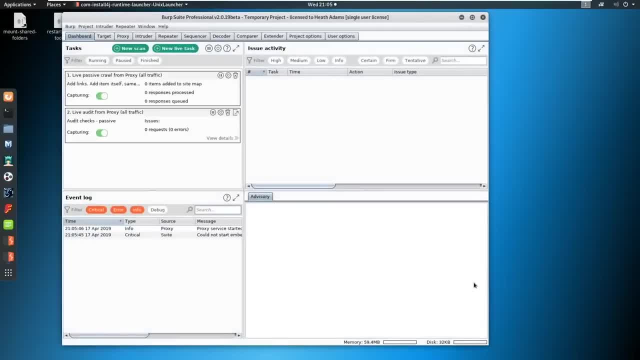 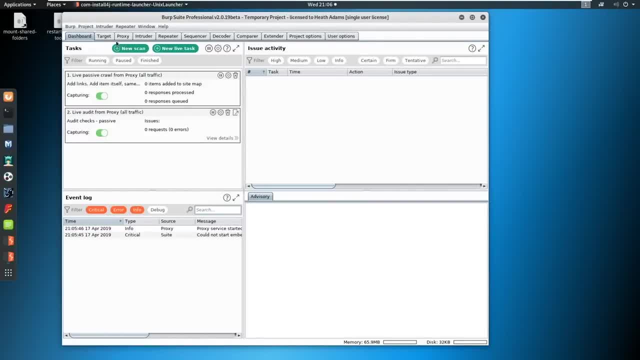 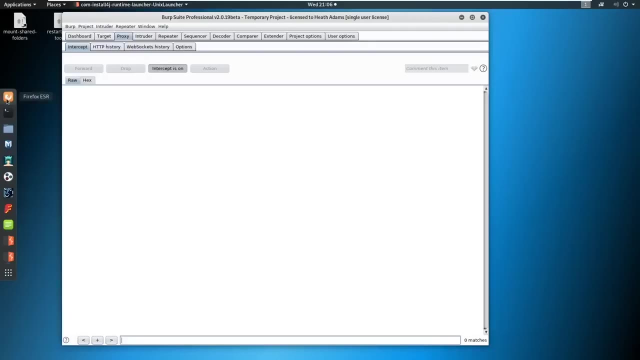 still trying to trying to decide, but I've been using it. um, on the last couple of assessments I've done these past couple of weeks and it's been fine. Okay, So we're going to pick a target, We're going to pick Tesla again and you can see, this intercept is on. Now we open up. 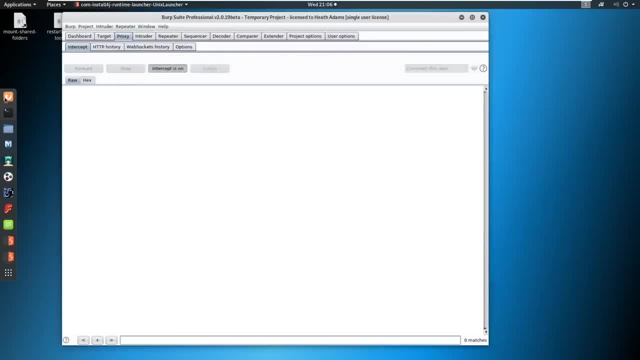 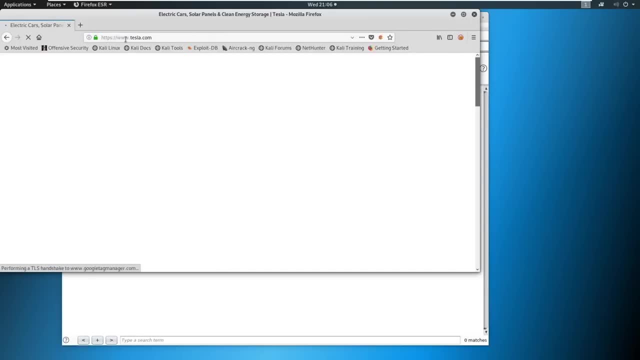 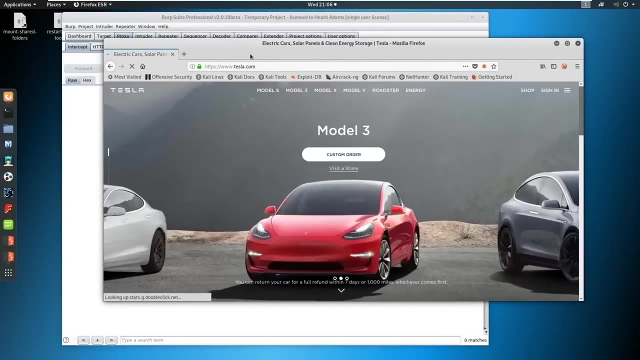 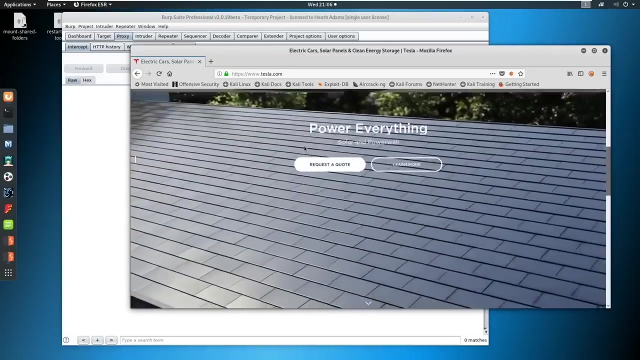 and we just say, okay, well, that's not what I wanted to have happen, Let's go to Tesla, We'll see what happens. All right, So we're on the Tesla website, but we need to make our browser talk to Burp Suite. Now you can. 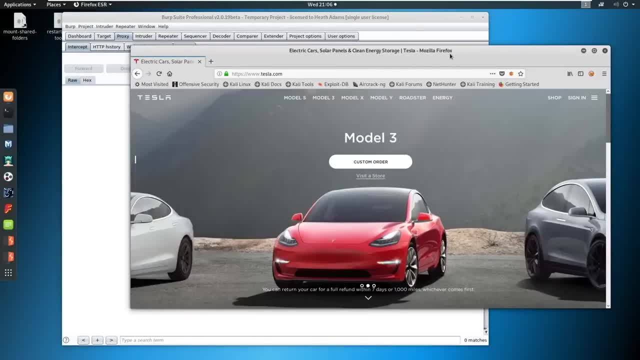 absolutely do this if you're trying to follow along or just you know, kind of get used to Burp Suite. This is important anyway. Um, I have a tool called Foxy Proxy here that I set up that just allows me to quick change into Burp. However, we're going to do it the old fashioned way, just. 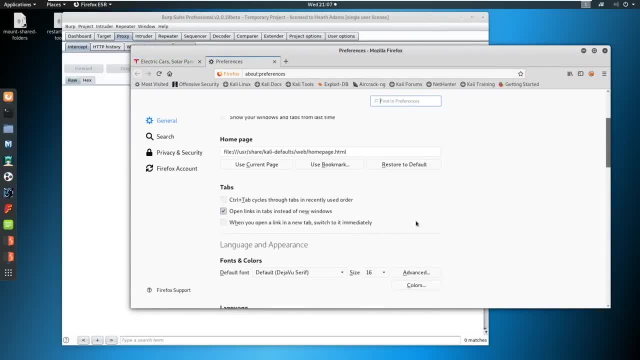 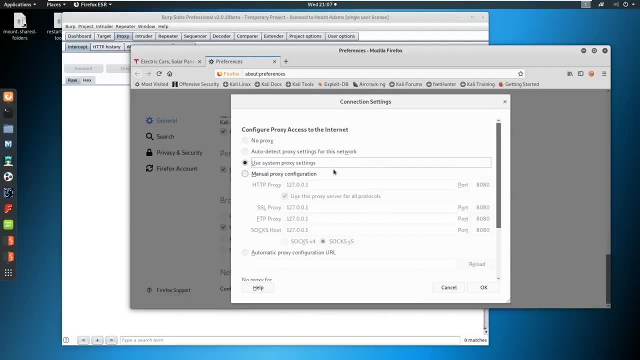 so you can see it, because you probably don't have Foxy Proxy installed. Um, if we scroll down all the way down the bottom, we're going to see a little bit of Burp Suite. So we're going to go to the bottom of the settings. We're going to go to our network settings. You're going to say: 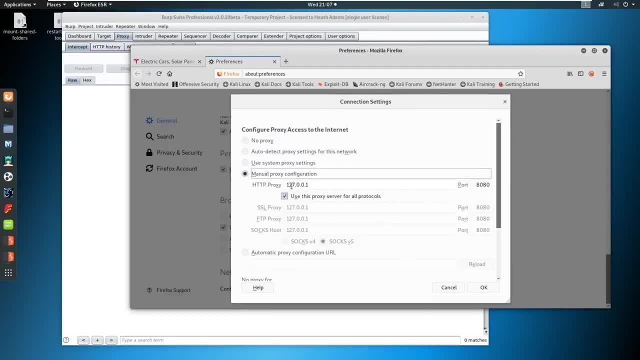 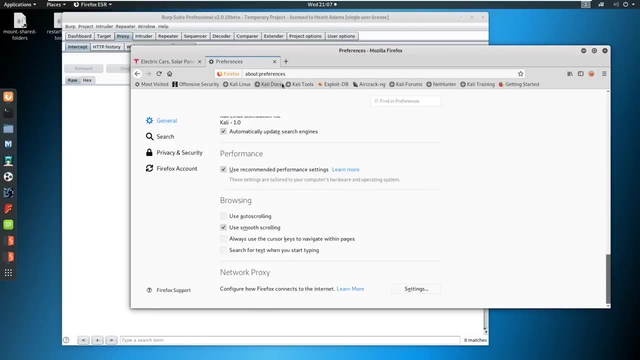 manual proxy configuration. Go ahead and use the home address of 1-2-7-0-0-1 on port 8080 and make sure it's set for all protocols. Okay, I'm going to go ahead and just use my Foxy Proxy to do that. 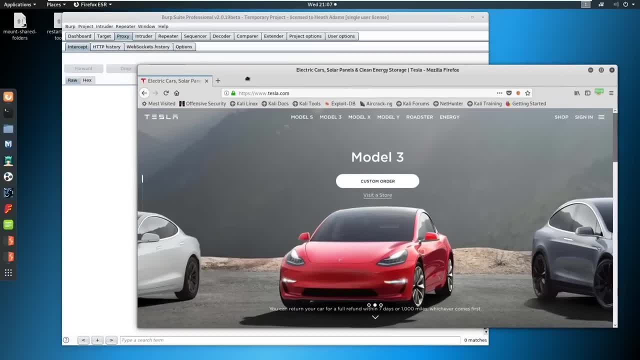 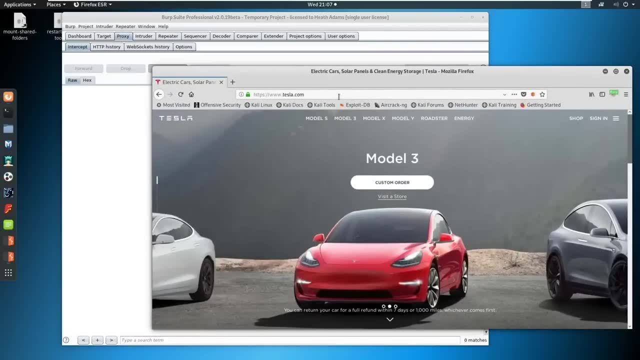 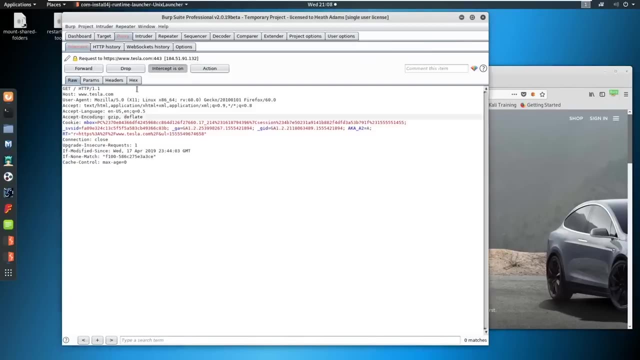 Okay, Now I've got this intercept on. Intercept on comes by default. You'll see what this does. Firefox is my preferred browser for doing assessments. Yes, Okay, So we're refreshing the page. You can see it's hung up If you look here. 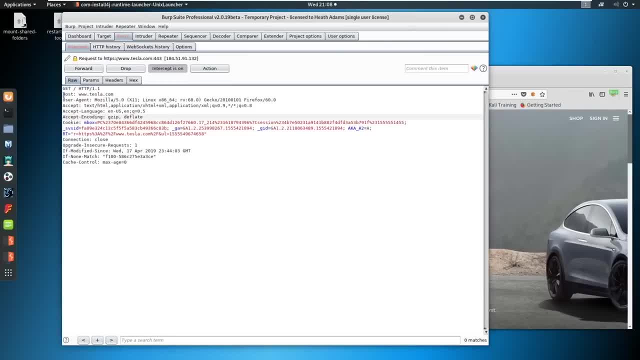 um, it intercepted the request. that's getting sent. You can see that it's a get request and I don't want to dive too much into this. I'm just showing you some of the very, very basics. Um, we And, as you can see, that we can get access to Divide with items if we want. Um, we have a lot of things. 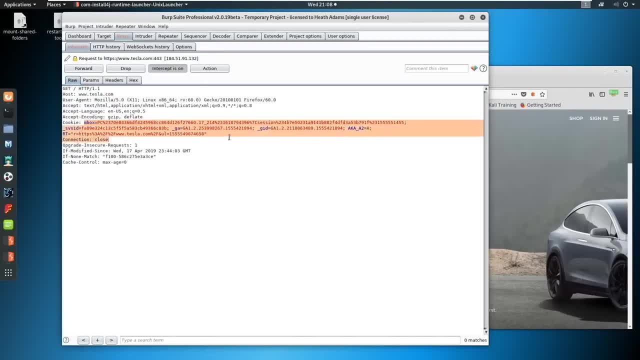 that were not bring anything into theitz. we have passer or theter support um trans appliance. we can do with this request. We can sit here and alter it. We've got these cookies that are kind of given to us by the site. We can try altering things that are here. You can see the user agent. 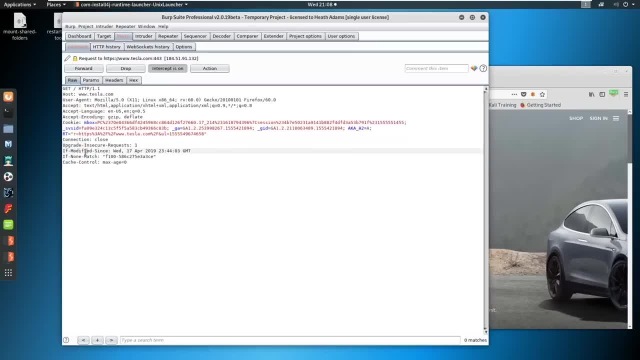 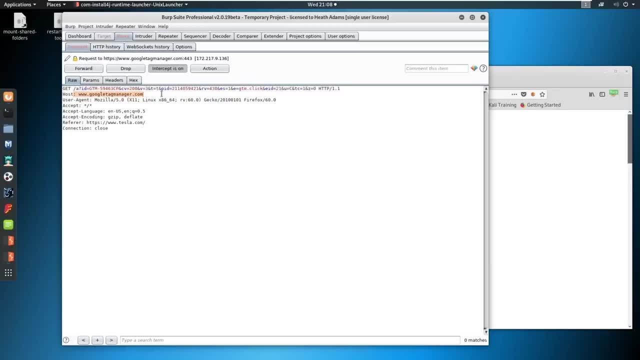 You can just see a bunch of header information and things like that. We can hit forward and see what happens. It looks like it's reaching out to Google TA or Google Tag Manager, if I could read for that. You can just keep forwarding. With a site like Tesla, there's going to be a million. 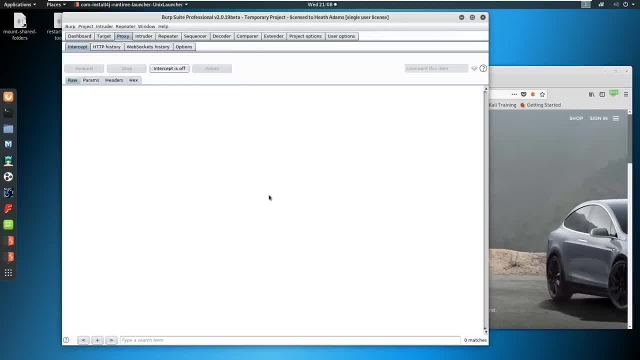 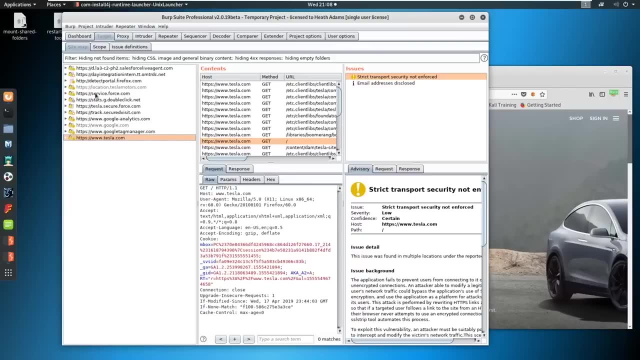 things. You can just turn the intercept off. If you come into Target, you can see a bunch of stuff in here that is loading in. Anything that is coming through from this site, it's reaching out. One of the most important things that we need to do is we need to right-click on the site. we 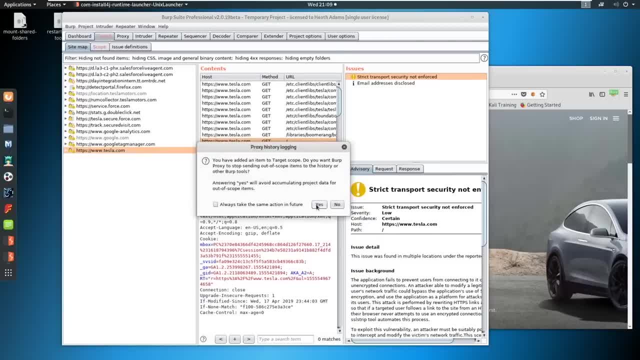 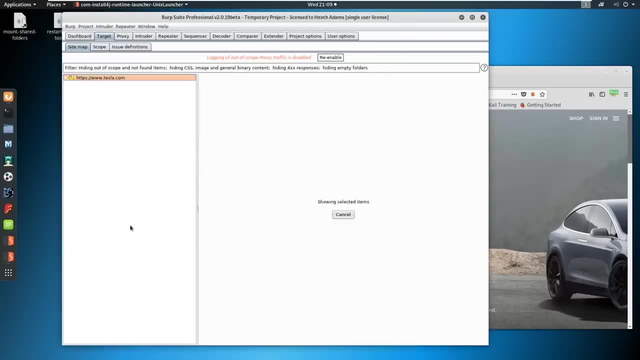 want to test and just say add to scope, We'll hit yes to that. We're going to come in here and we're going to click on this bar that says filter. We're going to say filter only in scope items. Now, Teslacom is our in scope item. We don't have 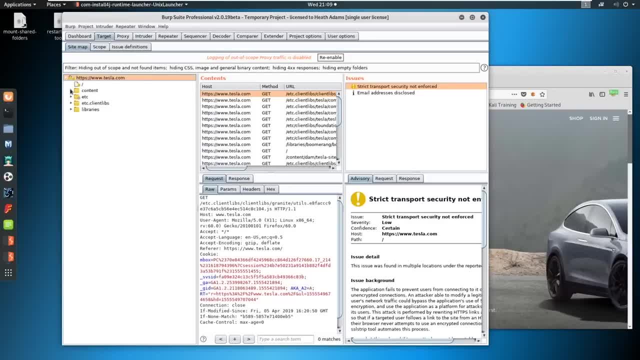 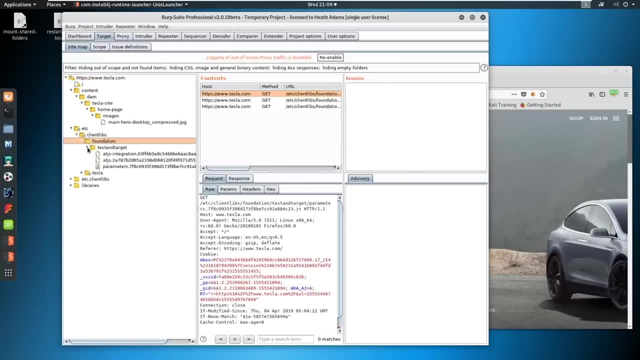 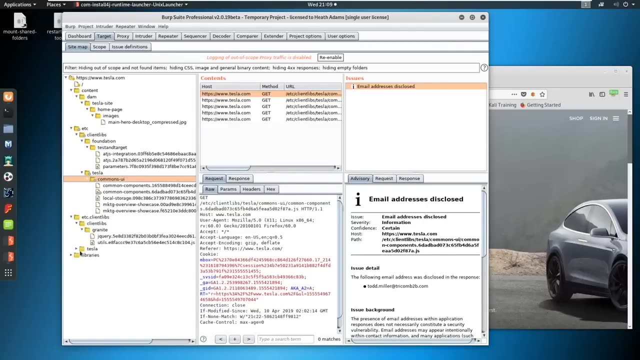 to look at anything else. Now, what you can see that it's doing for us is it's actually going through and kind of spidering passively. It's looking through all the things that it can find and it's even doing a little bit of scanning for us. You can just kind of come through here and 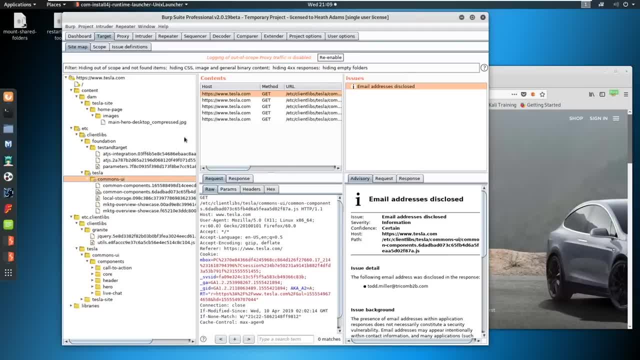 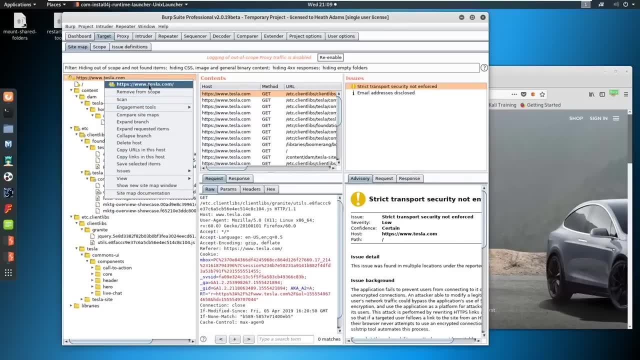 click on these things and find a little bit of information. Now, the old burp used to have a right-click and it would just say spider this branch. That is now gone. They have put that into the scan feature as well, but it is doing passive spidering by default, If you wanted to test more than just Teslacom. 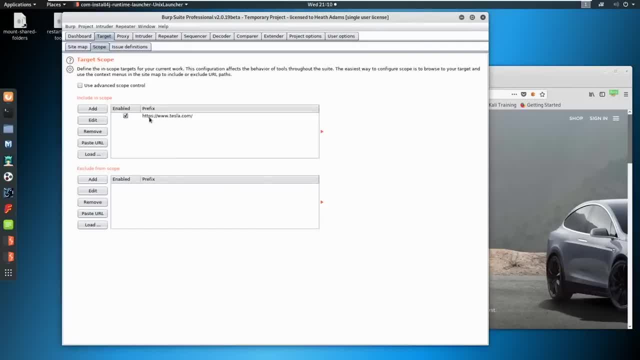 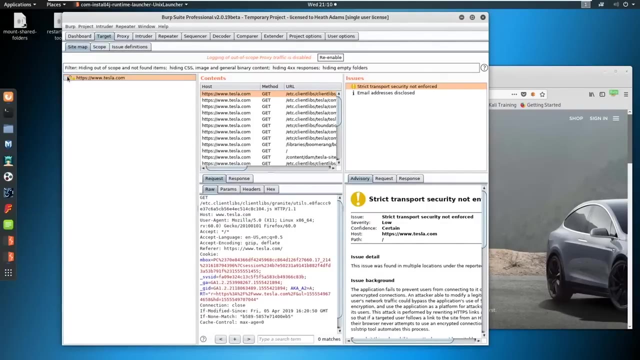 to your scope. there's some regex type feature that you can add to your scope. that would include everything as a wildcard here instead of wwwteslacom. This is starting to get a little bit more advanced and on the web app side, But the most important thing to know is that we want to make sure that we only scan what is in scope. 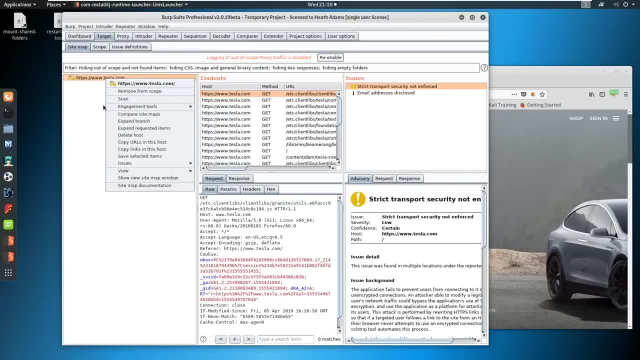 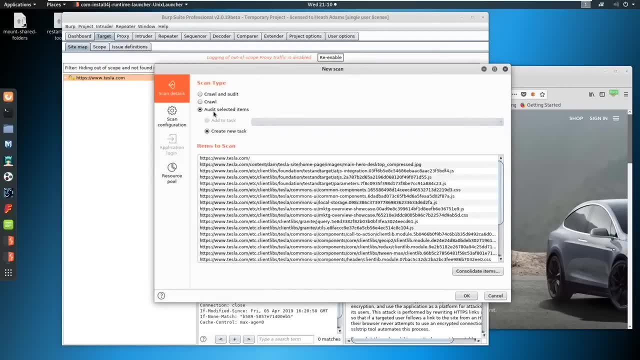 Yes, you'd have to check. use advanced scope control for that. All right, so we're going to scan here. You can see that you can do a crawl and audit. You can do a crawl, You can audit selected items. It gives you all the items that you want here. 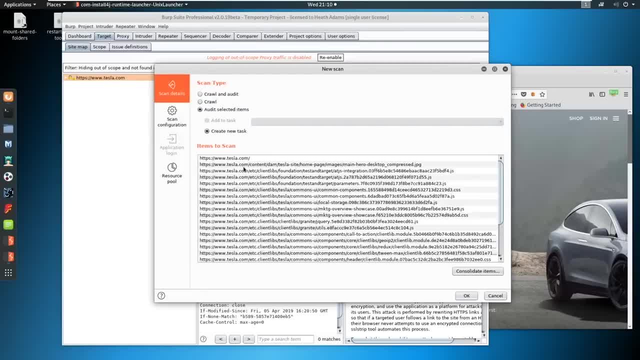 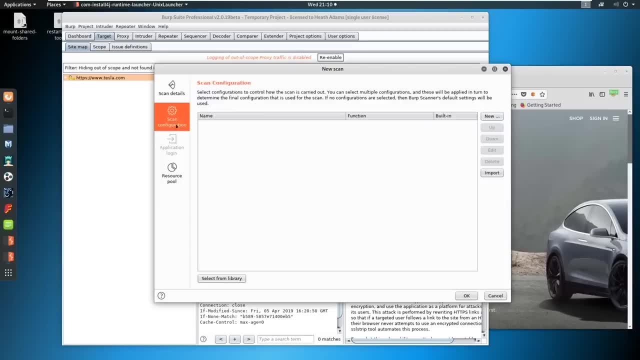 I just pick all of them typically, But if you wanted one specific item, just like Teslacom, just the homepage, you could do that. If we wanted to scan through everything here, we could as well. You have the option to configure your scan. You could set resources here. Depending on the website, 10 goes very slow. Sometimes I bump it up to 100, but sometimes it also makes things air out like crazy. So you need to make sure that the website you're using can handle the concurrent requests that you're doing. 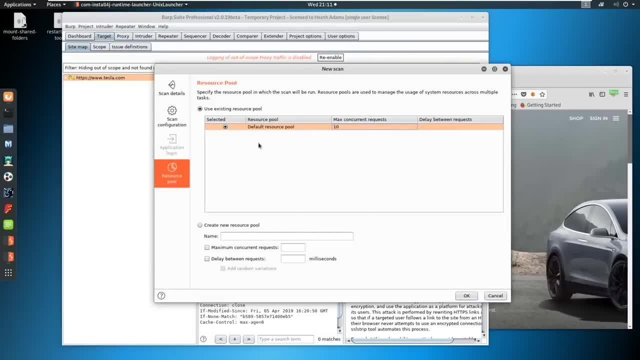 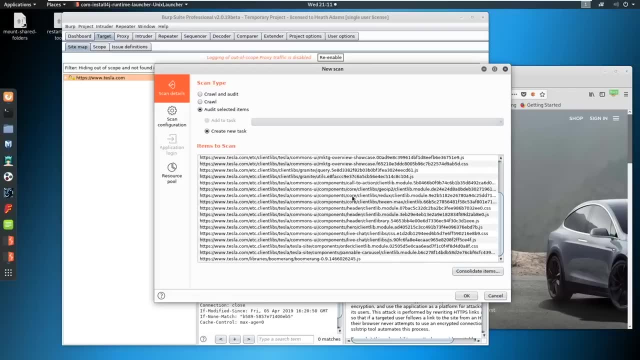 Or else it's just going to make you miss stuff. So 10 is fine as a default. But if you wanted to create a new resource pool, you can. But for very, very, very basic features we'll just select everything hit OK. 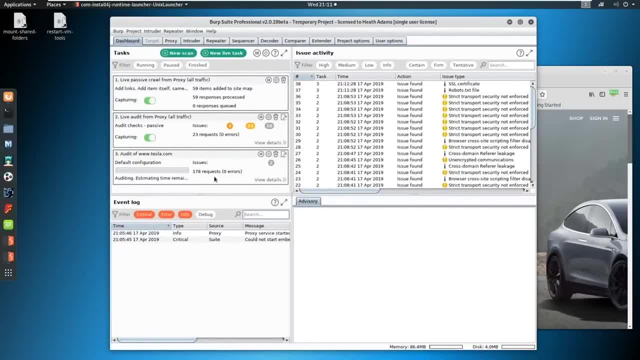 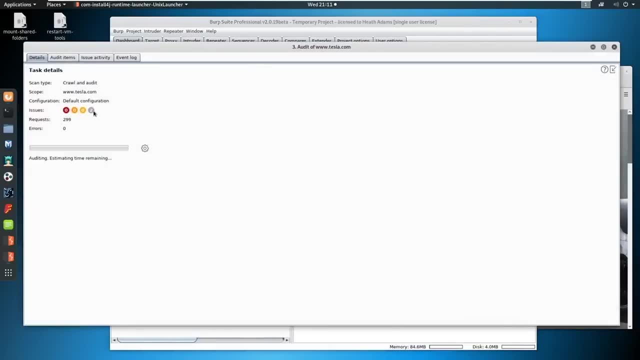 And we go to our dashboard and we can see that it is starting to scan And it'll start to pick up issues as it goes along. We can sit here and say view details. It looks like it's found two informationals so far. 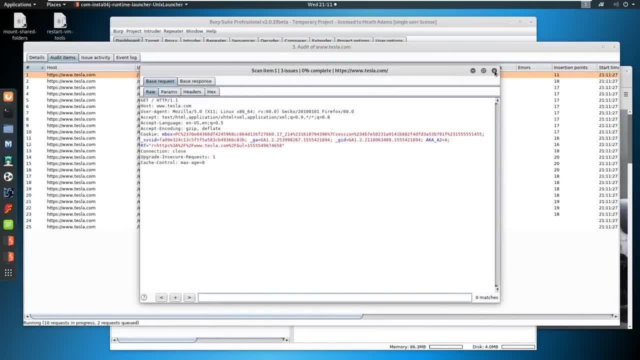 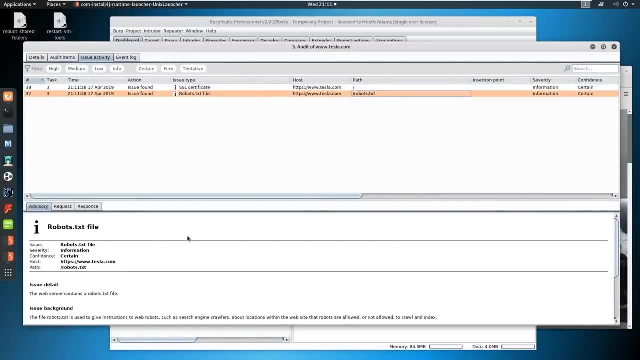 You can double-click on it. It used to have a better way of seeing the issues, but you have issue activity here. It found a robotstxt file. Those are always interesting, So you can see the request for the robots and then the response as to what's sitting in the robots. 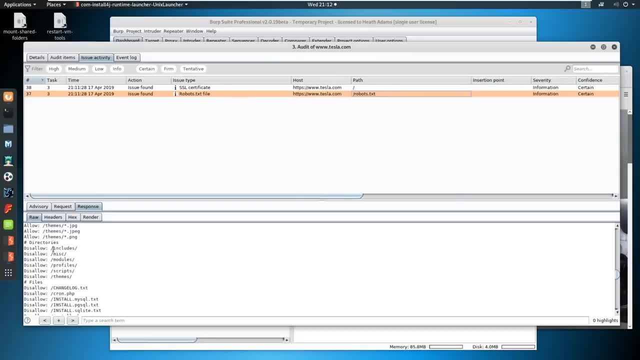 And then it has all the disallowed. So this gives you some directories. You can gather some information here if you're looking at the robotstxt. So you see there's an admin here, a slash admin as well. I don't know if that takes you to the slash admin. I don't know if that's in scope. 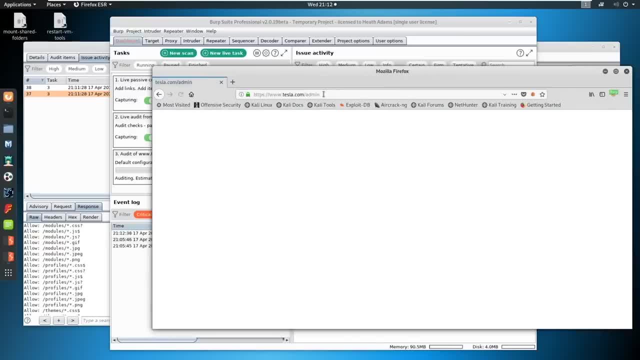 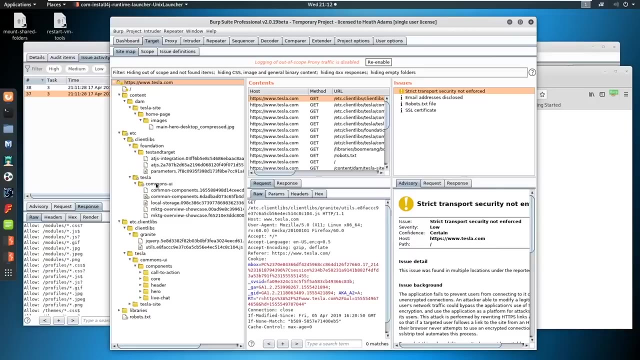 But they don't want you to see it on a Google search. So who knows what it does? Nothing there, But ideally you'd want to crawl the site first and try to crawl as much as you can and then scan it after you've crawled everything. 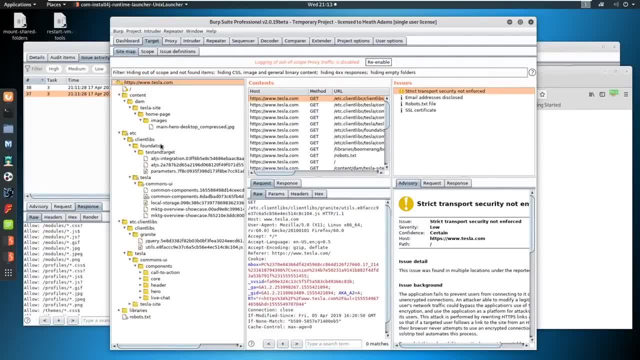 If I'm paying for share hosting, do I gain the right to scan my host provider legally as well? I don't think so. I don't think that's a yes. All right. So this is Burp. We're going to let that scan run as well. 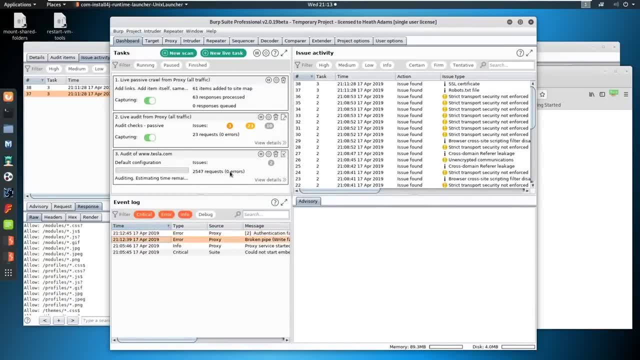 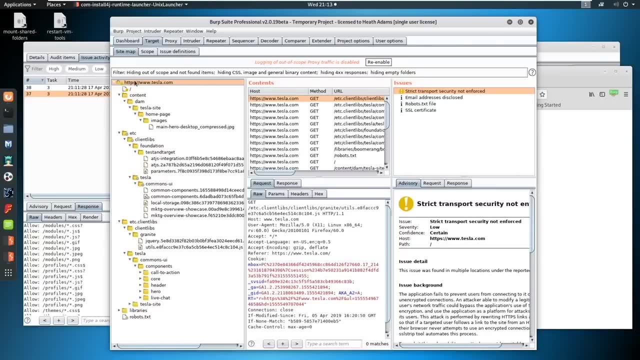 You can tell. sometimes there's errors that come through here. It doesn't even look like we have any errors on ours, So that's good. Everything is scanning fine. This will take quite a bit of time, depending on how many subdirectories and files that we scan. 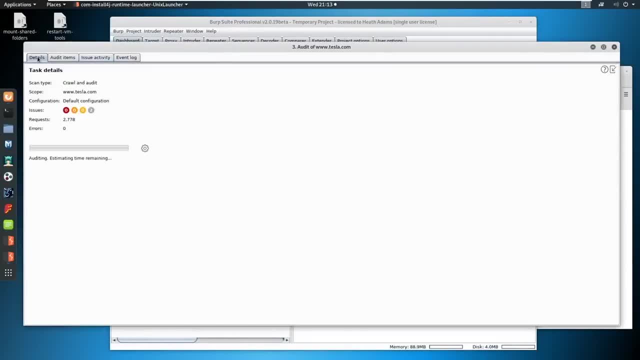 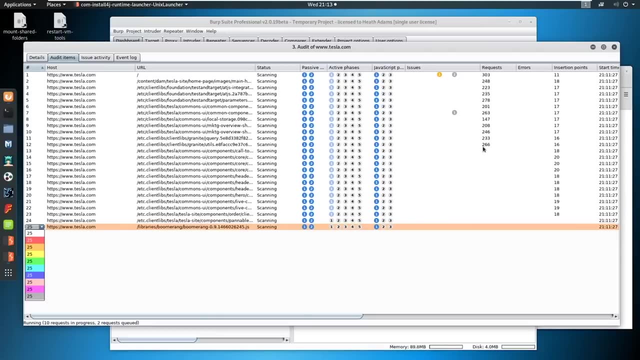 We really didn't scan that many. If we view the details again and we come back to the details of the odd items, we scan 25.. 25 is not really a lot. You can see that it's running 10 threads concurrently, like we suggested. 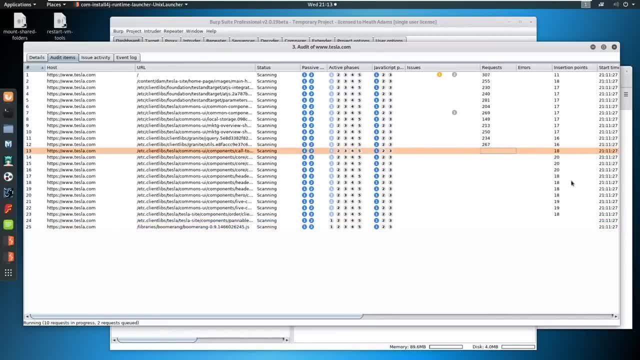 So once it finishes one of these, it's going to move on, Depending on the insertion points, like this, 11 insertion points, that'll be quicker, obviously, than 18.. So we'll let this run and see if we can find anything interesting in it. 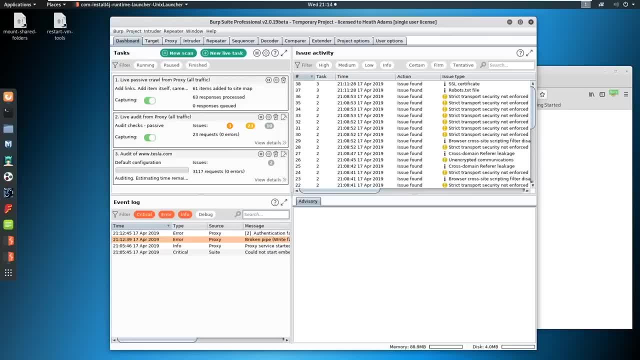 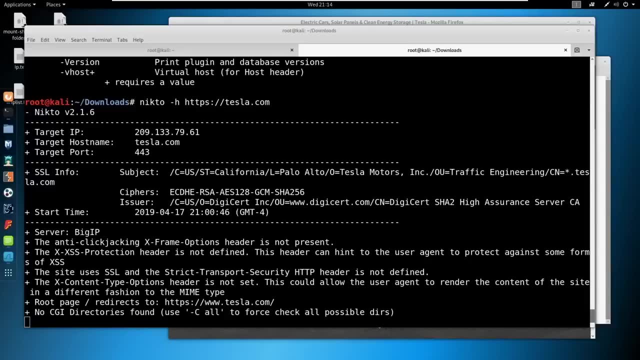 All right, Let's go back and check on our specific scans that we were running with Nessus and Nmap. All right, So Nicto is still running, Nmap is still running. We're down to 11 minutes, though That's pretty good. 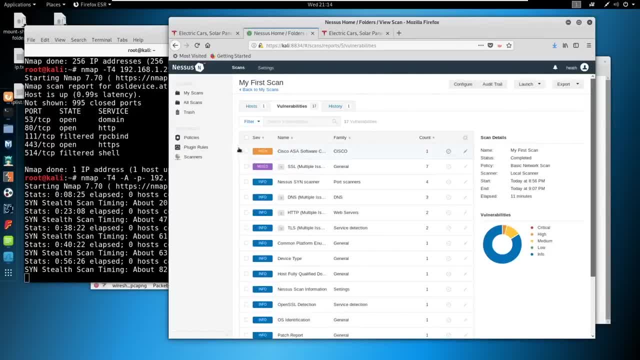 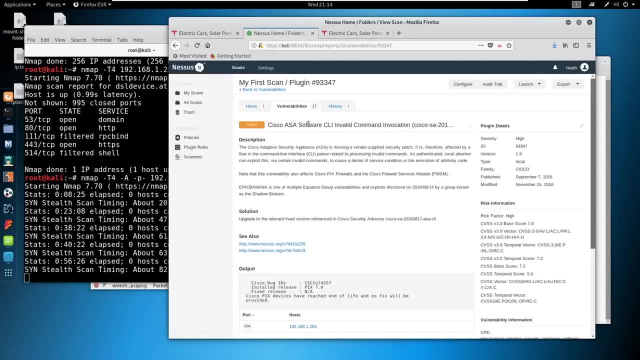 And Nessus- Oh, Nessus is finding some stuff. What kind of vulnerabilities do I have? What kind of vulnerabilities do I have, guys? It says I got a Cisco ASA software CLI invalid command invocation: Epic banana released by Shadow Brokers. 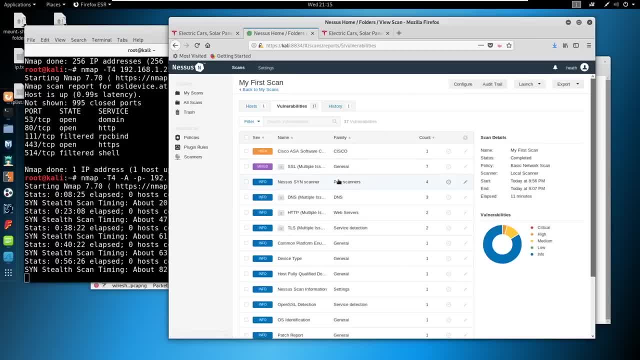 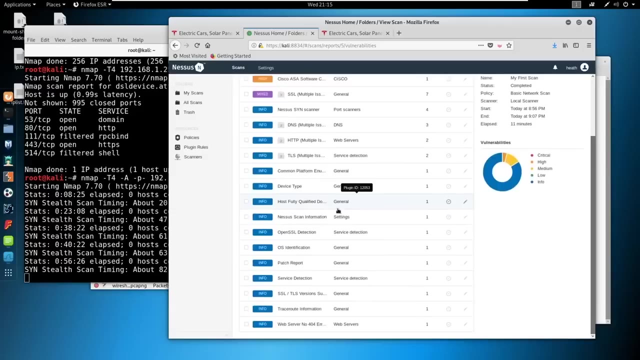 Good thing, I have no control over my router. It's got SSL information, DNS information, HTTP information, So let's see: Is this done? It's done. So basically, we would come through here and when we get to the enumeration phase. 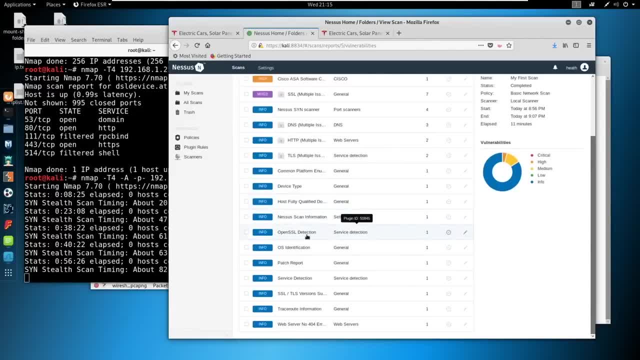 we would start looking through this and seeing what we can pull out As of right now. we're just trying to gather as much information as we can. It's got a fully qualified domain name. It's got OS detection. That's interesting. 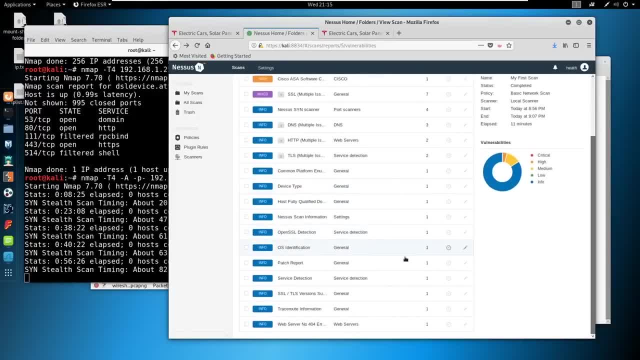 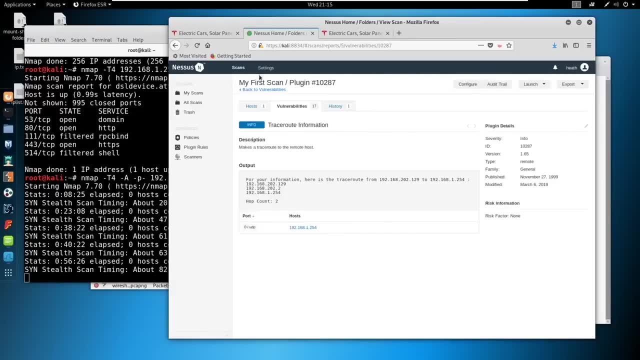 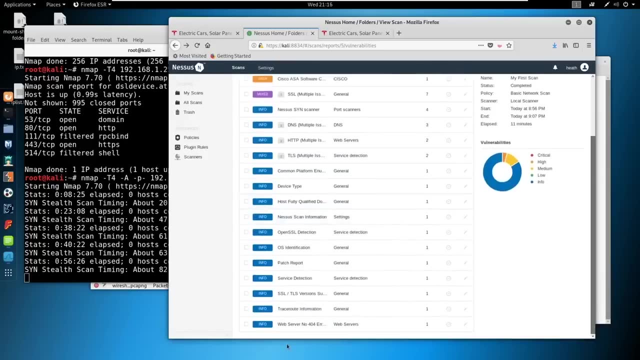 It says it's running. It's running Cisco Maybe, Service detection 443.. Yeah, 443 is open Trace route information. So this is what we would do: We'd come in here and look and we'll talk about enumeration next week. 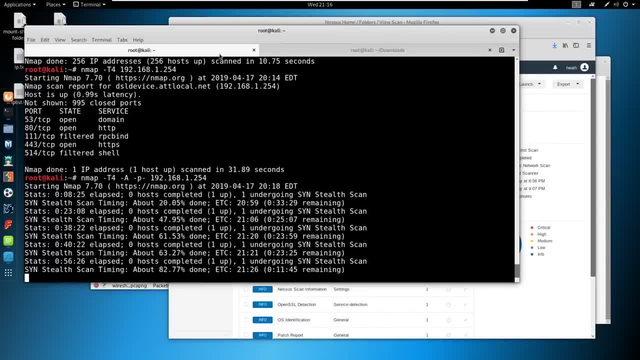 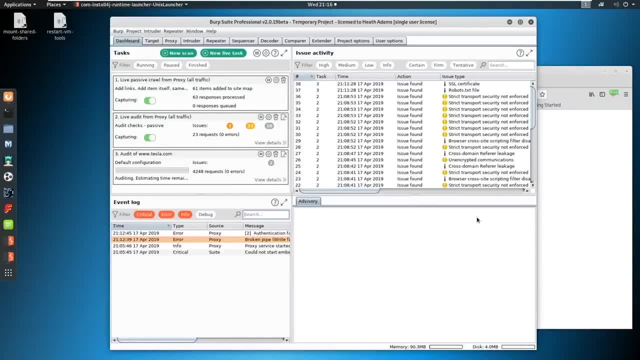 So we're going to wait on some of the scans. I will let them come. They're going to come back up as they go. I think I'm going to go into the Q&A early and then we'll come back and hit on some of this stuff. 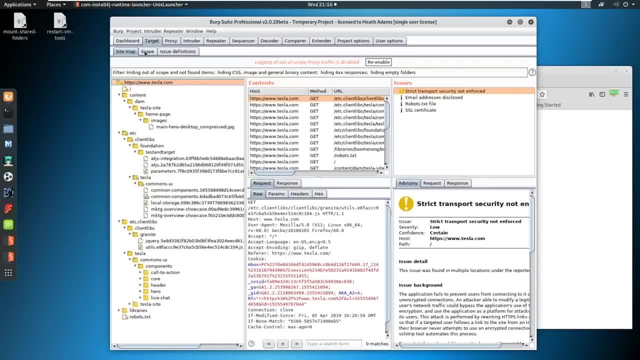 since nothing's really happening. I'm not expecting to see a lot from Tesla either, so I'm sure they've been picked pretty clean, but we'll see what comes up. So I'm going to switch over to the live scene and we can do some quick Q&A. 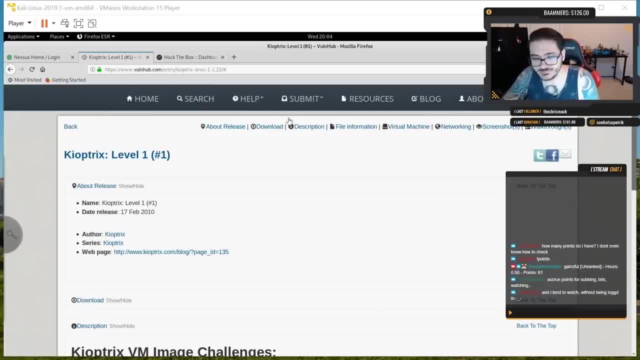 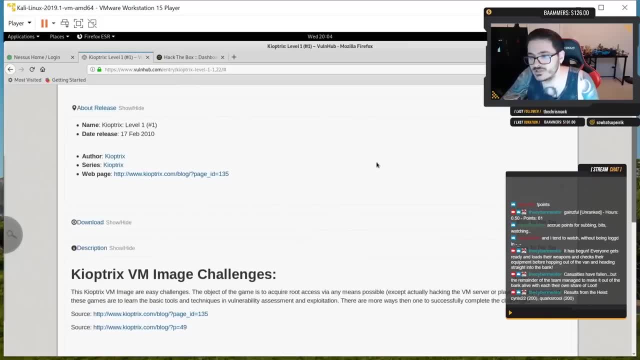 So we are going to be scanning Keoptrics Level 1, which I sent out an email that you guys needed to be downloading. So if you've got Keoptrics up, it should have if you're. I'm running a VMware player. 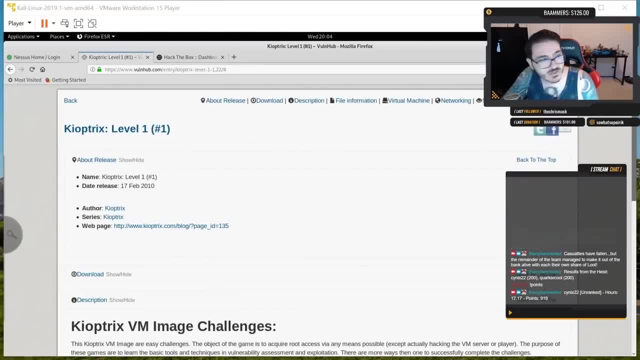 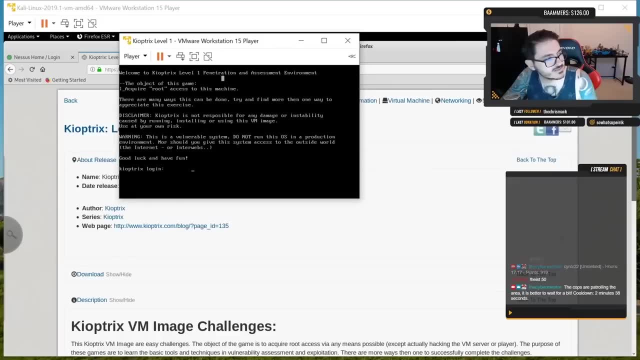 so that I'm running the same as you guys. You should have two players open. essentially, If I drag this over, your Keoptrics should look something like this where it says Level 1 Penetration, Testing and Assessment Environment. You got the Keoptrics login. 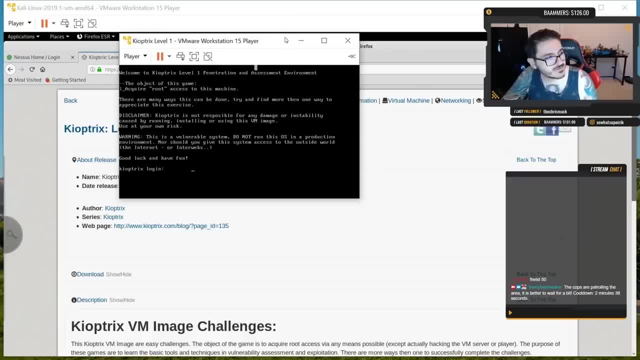 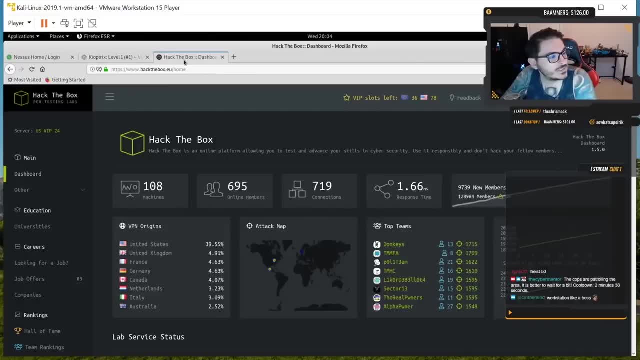 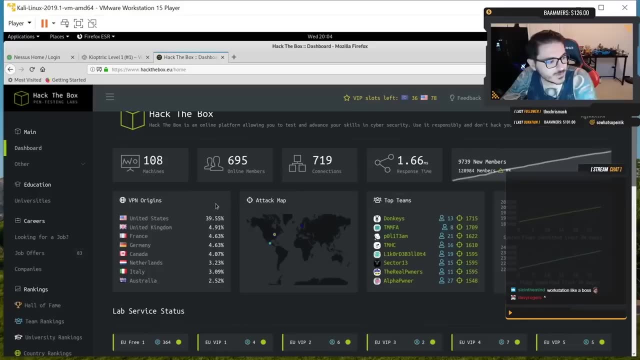 and you're stuck in this box. You just hit Control-Alt at the same time to escape. After that, we're going to be going into Hack the Box and we are going to pick a random box out of here, If you've never used Hack the Box before. 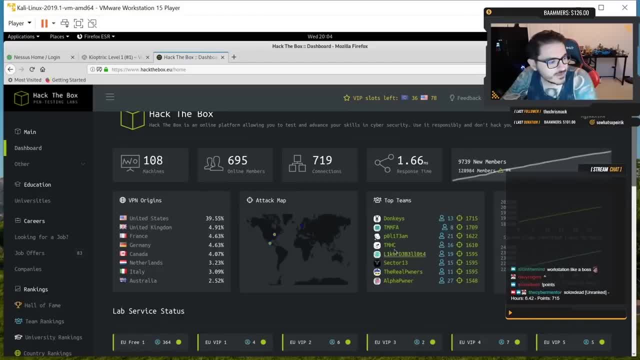 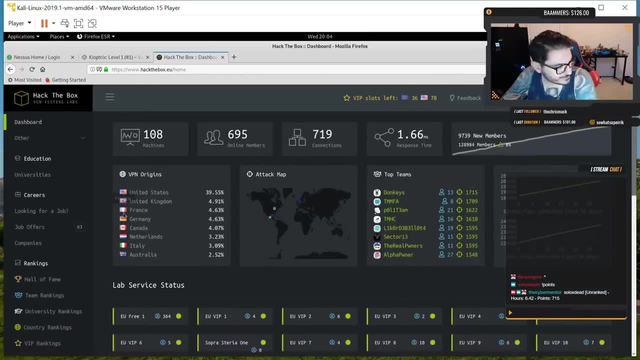 then this may be something for you. Hey look, Davy's team's up here in the top teams. Congrats, Davy. I didn't know that, So anyway, we'll come into here. We're going to Access. 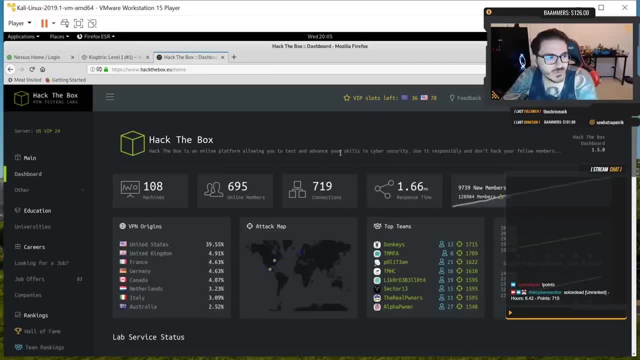 I'll show you guys how to do that. if you've never done Hack the Box before, If you haven't signed up for Hack the Box, you're probably not going to be able to do it tonight. It does require a little bit of hackery to get in. 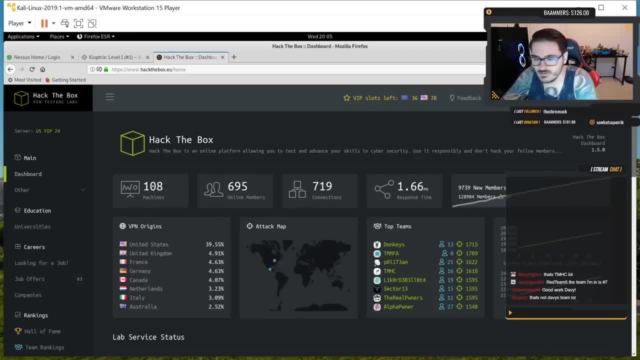 but that's okay, You can work on that in a later time. Just follow along with what we're doing and the reasoning behind it. So tonight we're going to be talking mainly about enumeration. Enumeration is the most important thing that you're going to be doing. 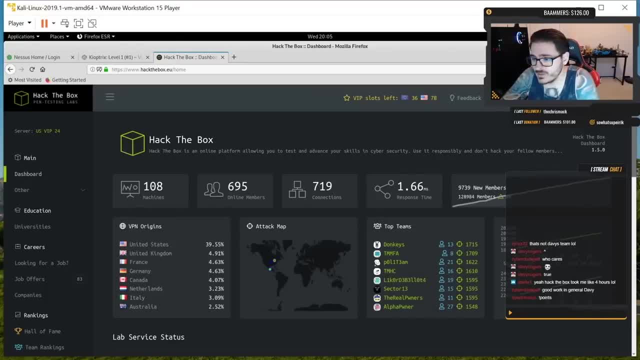 in anything hacking-related. So if you don't know how to enumerate, if you aren't patient with your enumeration, you're not going to be a good hacker and you're not going to be successful in the field. That's not your team. 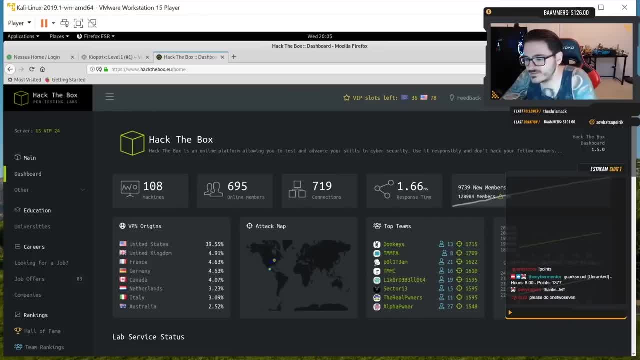 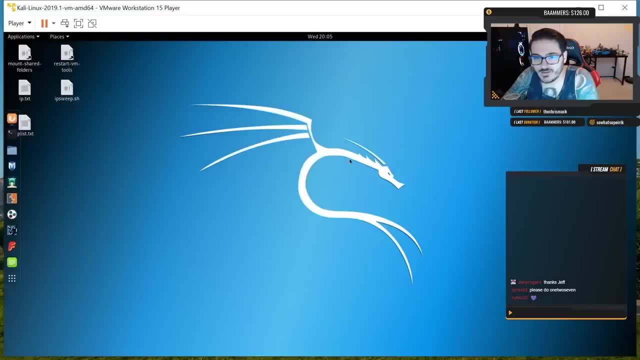 I thought that was your team. My bad, Sorry guys. All right. So, as I was saying, you won't be successful in this field if you don't know how to enumerate, So this is why we're taking it in baby steps. 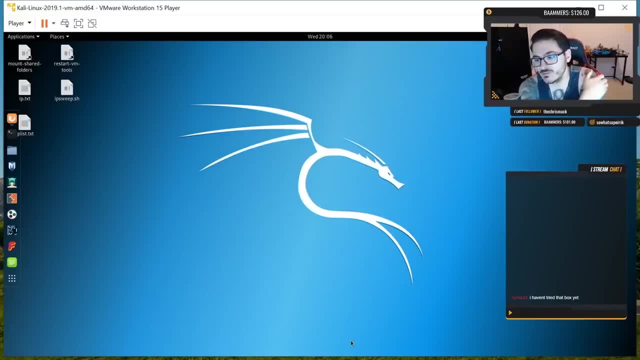 Last week we talked about scanning. This week we're talking about just enumeration. We're not going to dive into anything exploitation until at least next week. That way you can kind of understand what the process is Now. I'm not going to show you tonight. 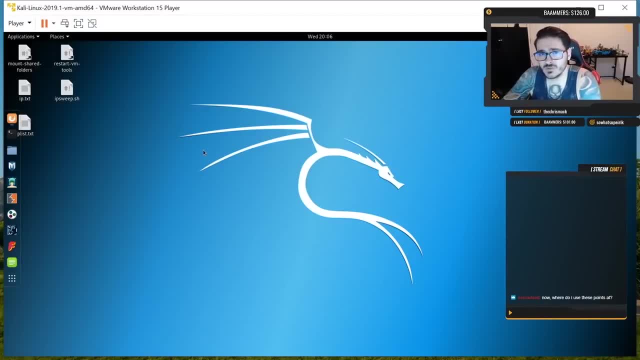 how to do every single port, how to enumerate what tools those are. I'm going to leave that up to you. That's your challenge is to go figure out how you would enumerate certain ports. I'm going to show you my process. 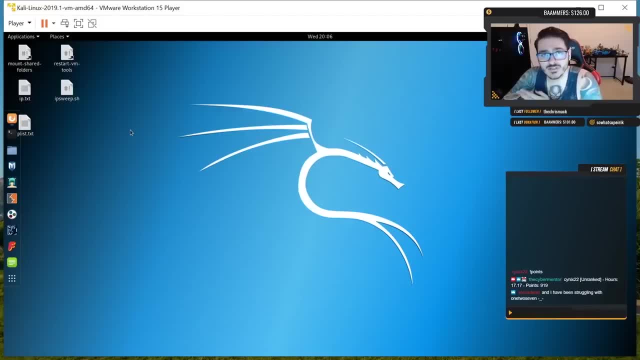 which holds true for any port that I'd be looking at, Any service, et cetera. So with that process you should be able to take that and move on and do any box that you see, at least from an enumeration aspect. 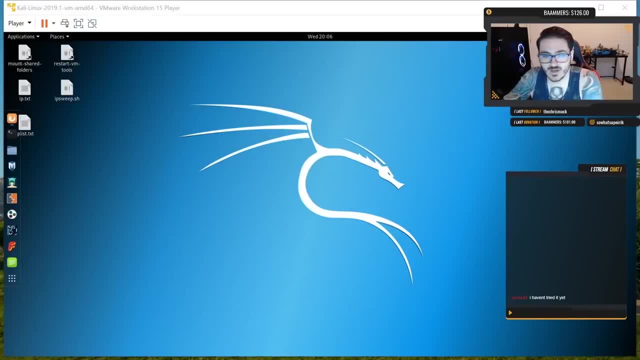 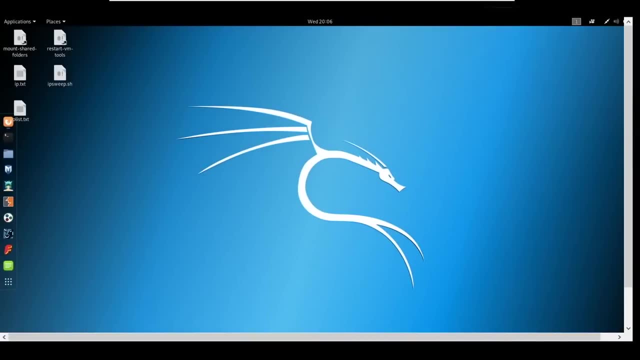 All right, So let's go ahead and get started. I'm going to take myself off of this screen. I'm going to make this full screen here. Okay, And now what we're going to be doing? first and foremost, we're going into a terminal. 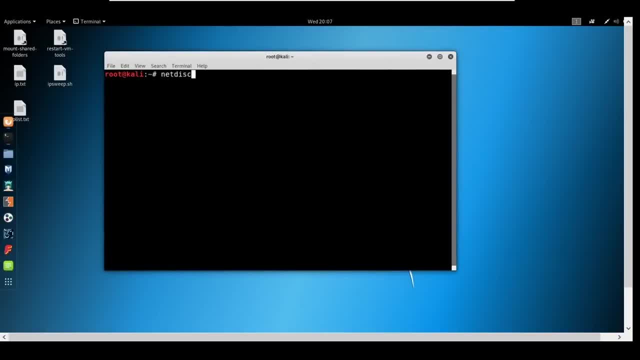 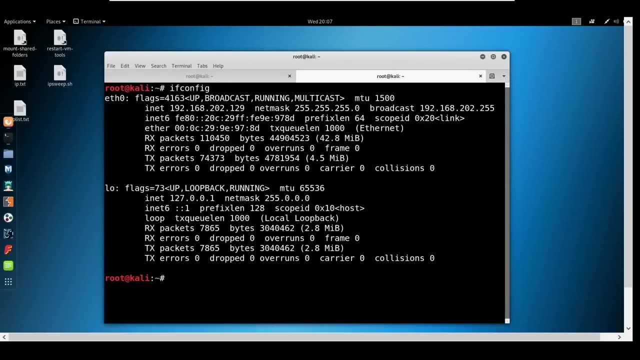 And we are going to do a net discover dash R. Also, I need my. I need a new tab here because I don't know my IP address. So we'll say ifconfig, Let's find your IP address. So my IP address is 192.168.202.129.. 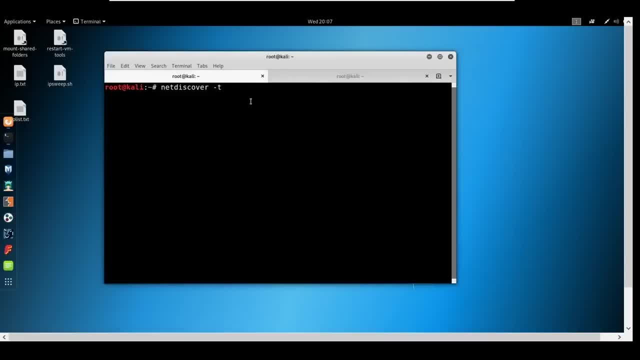 I'm just going to copy the first three octets. We'll do a dash R for range Paste 0 slash 24.. If this does not make sense, we are doing a discovery via ARP through this range. That's what dash R is for. 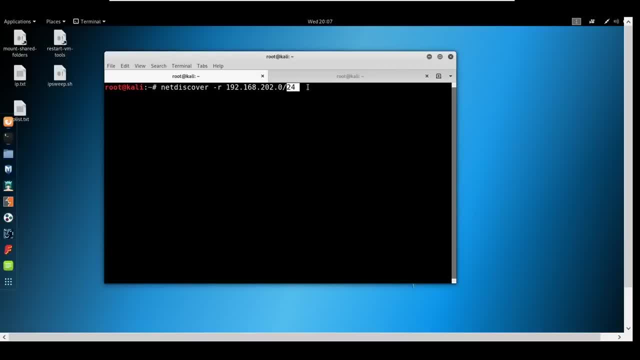 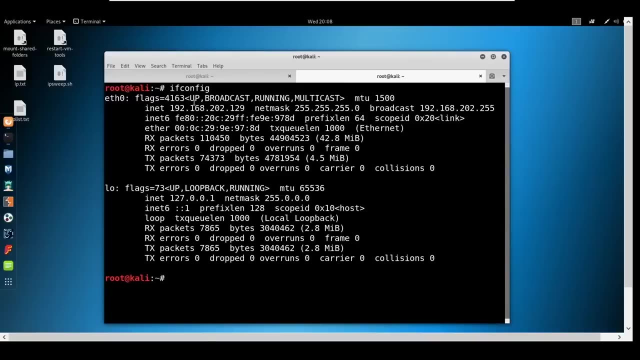 We're specifying a dot zero and we're scanning the entire subnet of a slash 24.. If you are weak on subnetting or understanding what this is, you may need to brush up on your networking skills. So we're doing the sweep. Remember that my IP is 129.. 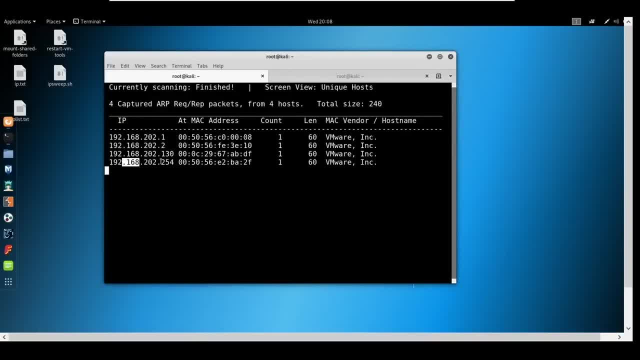 I expect dot one and dot two to be active. I expect dot 254 to be active. Those are active by default, But the one that really stands out to me is this: dot 130.. So this is our Keoptrics machine. 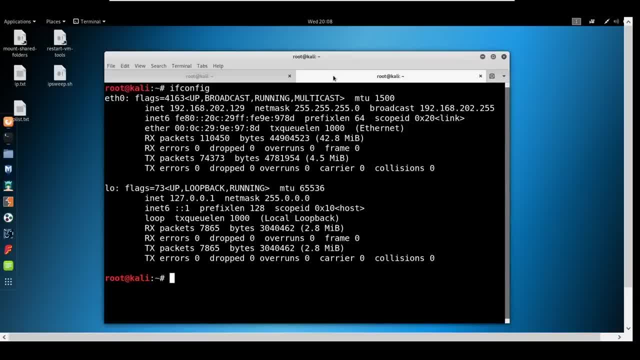 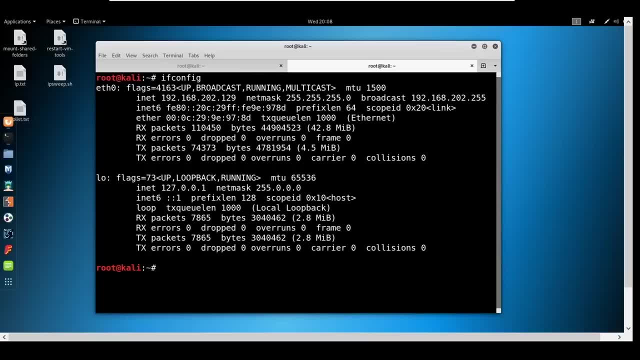 At least this is my Keoptrics machine, So I'm going to show you this Tonight, from my perspective, how I would focus on this machine if I were a pen tester. I'm not going to focus on this as if it were a capture the flag. 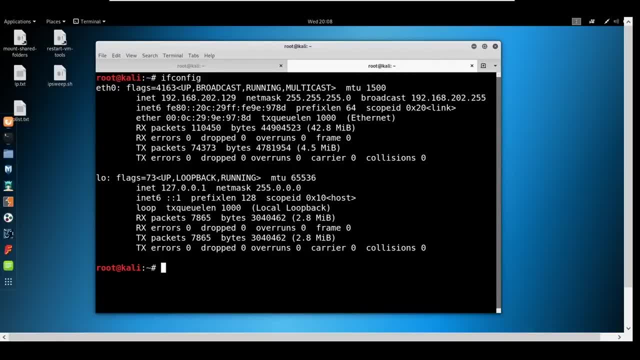 I want to talk about all the details that I would look at and what I would be seeing. We're going to talk about how I would report findings, what findings I would report, at least up until a certain point, before we even exploit anything. 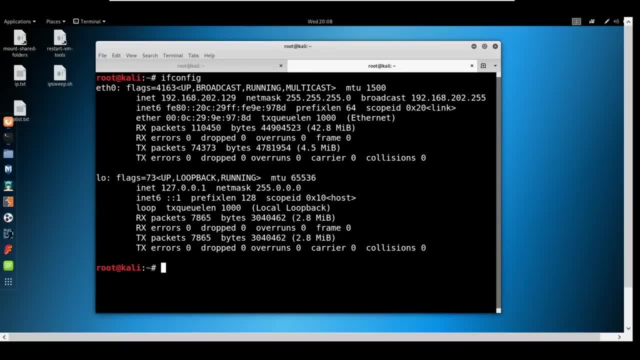 So there's a lot of information and details that you can gather without ever having to run an exploit. Another thing, another thing that you should have up for tonight is that we're going to be running our Keep Note. If you've got Cherrytree, that's fine. 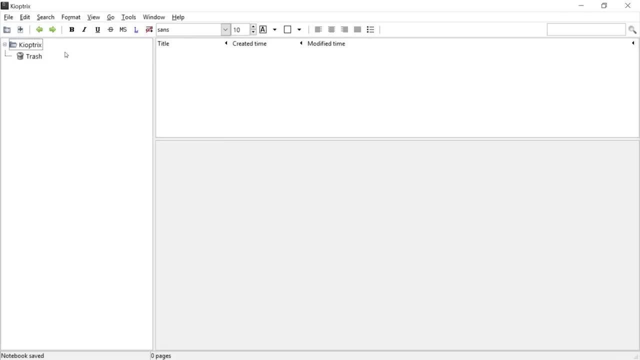 I've started a brand new Keep Note for Keoptrics. We're going to do it like I would do for work in a work-related setting. in the sense that this is going to be, we'll call this probably an external assessment. It could more likely be internal assessment. 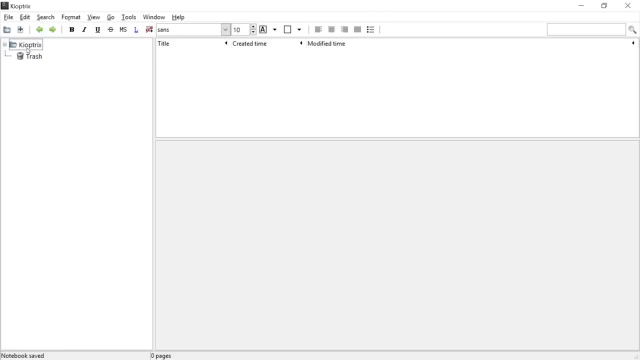 but we'll just we'll write it out where we create some subcategories here and we actually take screenshots And notate exactly what we're doing. That way we take good notes and we have something going forward. So that way you guys have notes later on in the class. 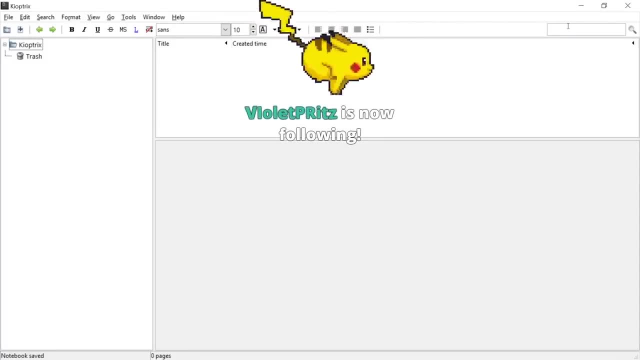 Somebody asked if you booted your Keoptrics VM. do you just need to leave it, or do you need to log in and do something with it? There is no login. You just need to leave it. We're going to try to hack it. 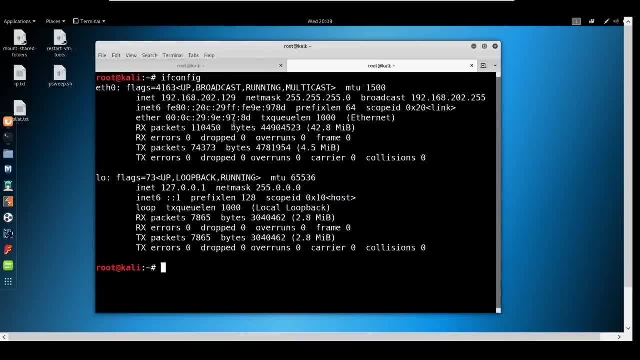 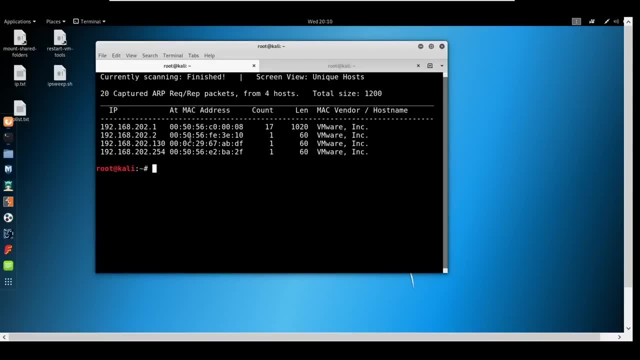 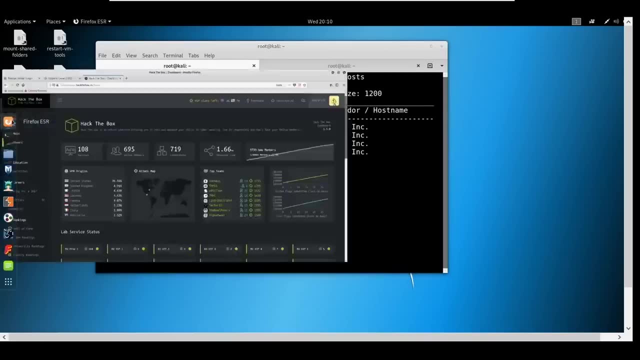 So good question, Okay. So, as a pen tester, we're going to do a couple of things, and we covered this last week. First and foremost, we're probably going to be firing up Nessus, So let's log in to our Nessus server. 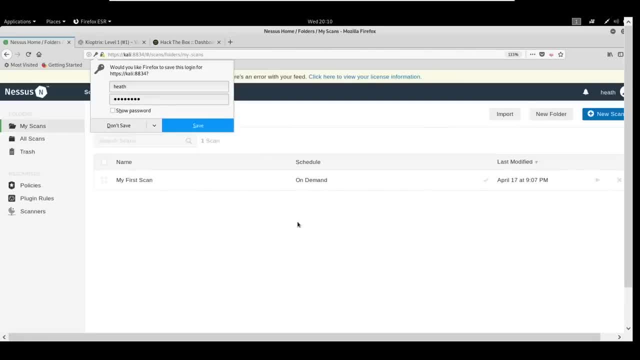 If you installed it last week. if not, then go back and look at how to install Nessus and run that. You can just follow along from the Nmap portion of it. So we're going to do a new scan, We're going to do a basic. 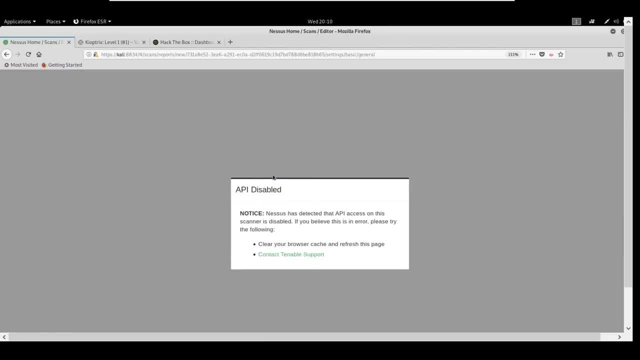 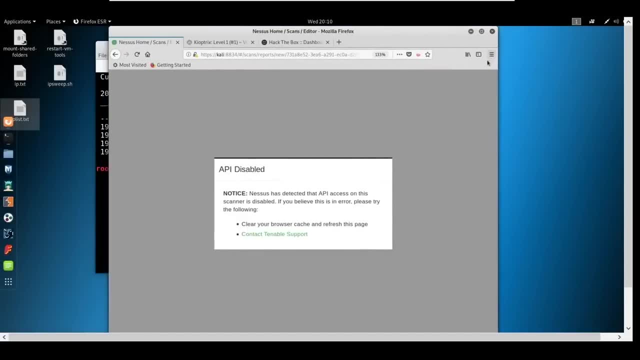 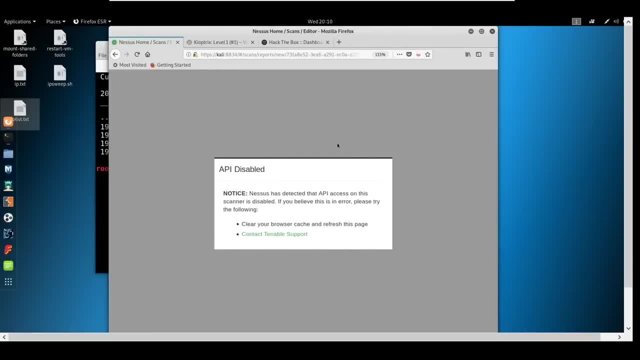 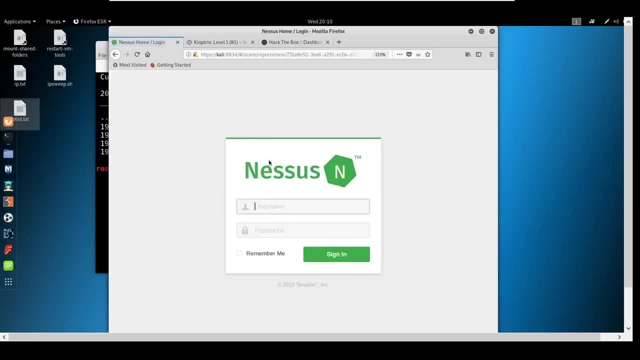 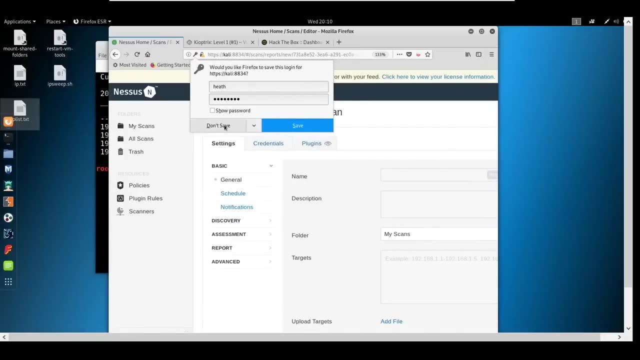 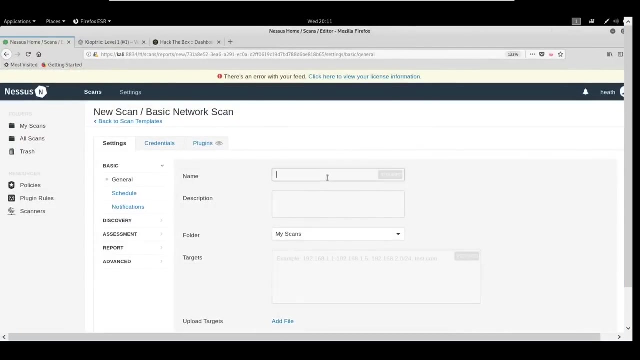 Let's go ahead and do a basic network scan. Let's go ahead and do a basic network scan for nessus. no, we didn't pay for nessus. this is a free trial which allows you to do up to 16 hosts at one time. so actually paste the ip there. we'll just call this keyoptrics. we'll call this. 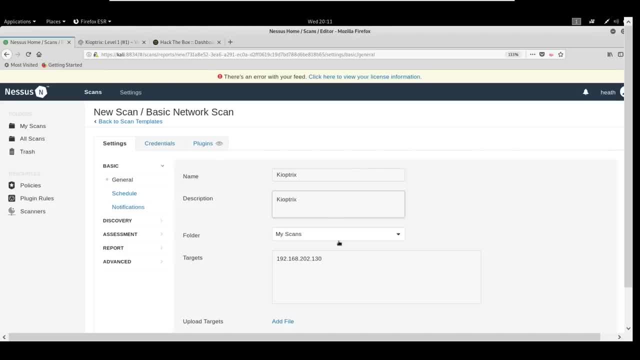 description, keyoptrics as well- and what we're doing is we're going to come into discovery. we're going to select port scan. all ports go into assessment. we'll leave assessment default. we're not going to scan for all web vulnerabilities. we'll scan for known web vulnerabilities. how about that? that'll be quick. 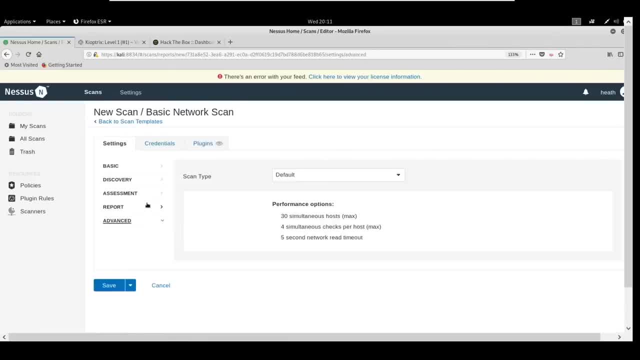 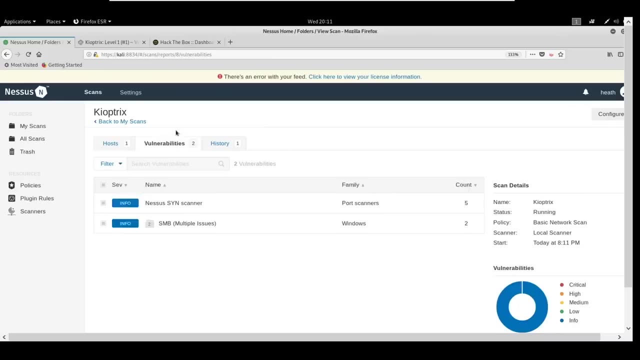 and then reporting's fine, advanced is fine, we'll save that and we're just going to go ahead and hit launch. and we're going to go ahead and hit launch. we're going to let this run. we can click on it and kind of watch it go as it picks up. 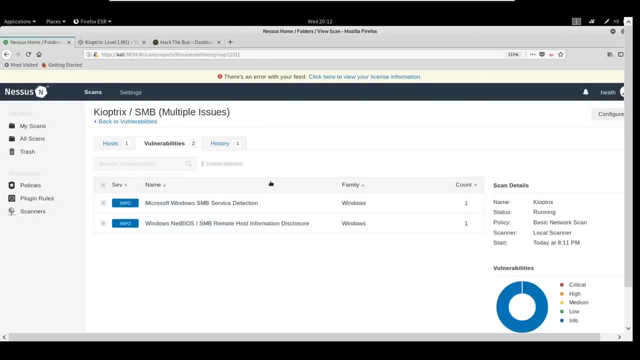 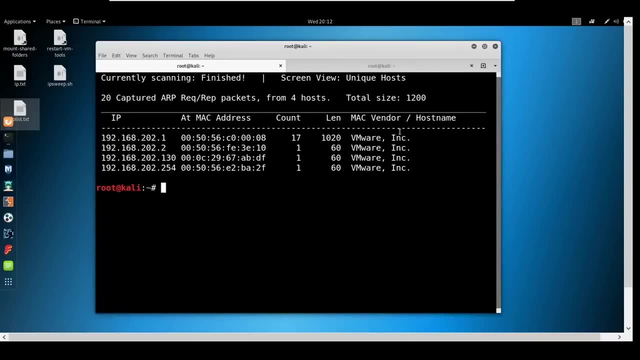 vulnerabilities or or other issues. so you can see it already. it's picked up, smb. we'll let this run while we um, while we go and do our nmap scans. so let's minimize that. let's go ahead and take a look at nmap. now i'm gonna make this one more bigger, okay, and we're going to nmap this guy. we're just 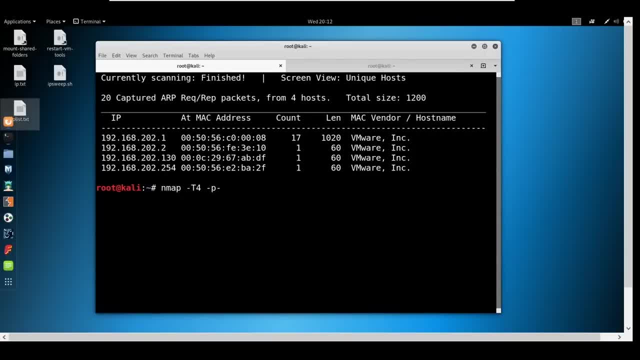 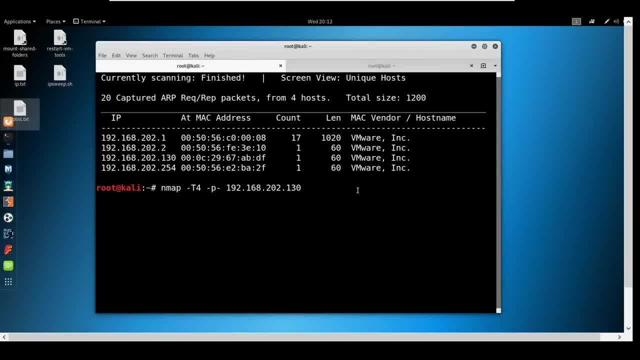 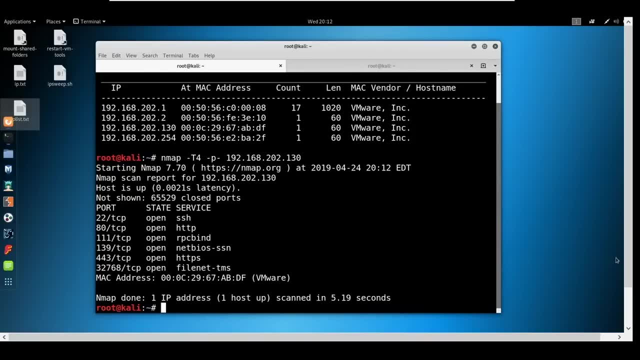 paste. i do okay. so we're going to enter in the ip address and just hit enter. now does anybody remember from last week what i'm doing here? can somebody tell me what i'm doing here? just as a little q, a reminder: what did i leave off and what did i leave off intentionally is the question. 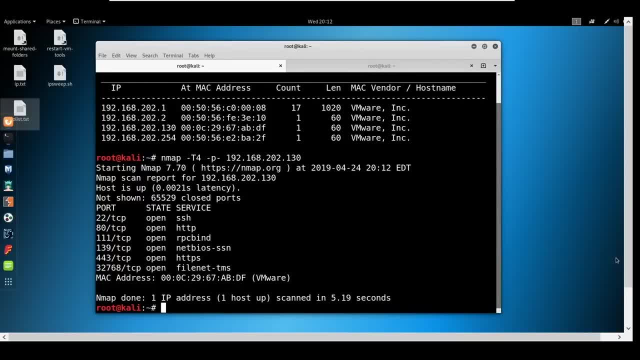 yes, i'm running nmap scan. thank you, gray. yep, we left off. we left off the a, thanks jake. so intentionally left off the switch of a. we don't want to scan for all on all ports, we want to do some stage scanning here. so now that we have this information we can tab back up. 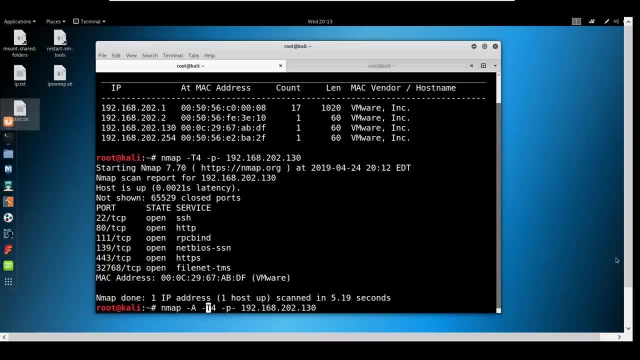 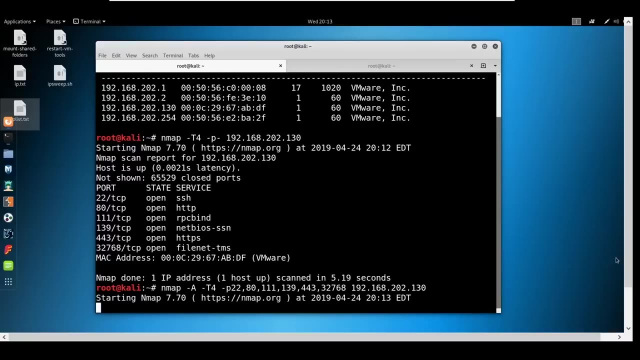 we can come out wherever you want to put it, dash a, and then you can put your ports in here, that you found something like this and i'm going to hit enter on that and we'll let this run. it shouldn't take too too long, because we are in a direct network and this is um. 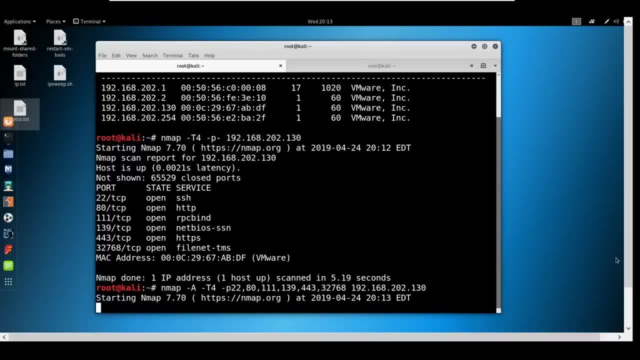 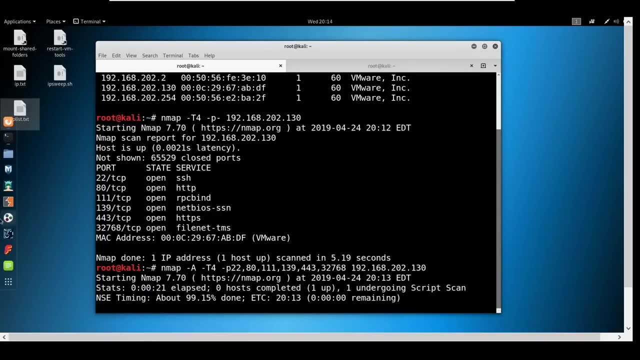 not scanning, say, a website over over a network, for example. so we'll wait for this to. to populate, let's hit the up arrow 99 on the nse. we'll check in on our nessus as well. oh, we're getting all kinds of fun stuff. 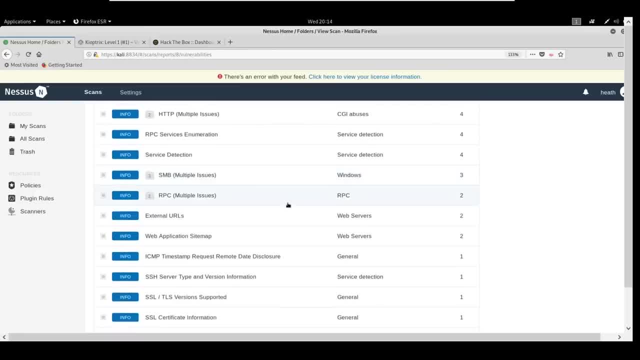 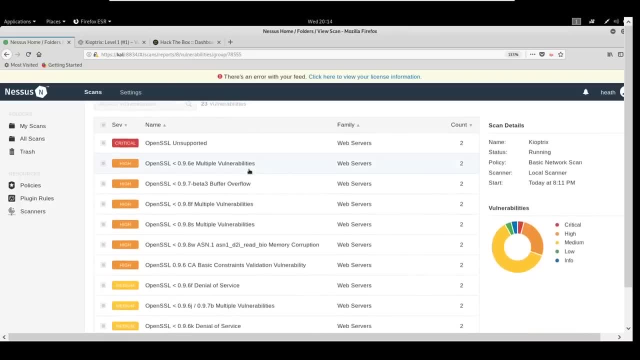 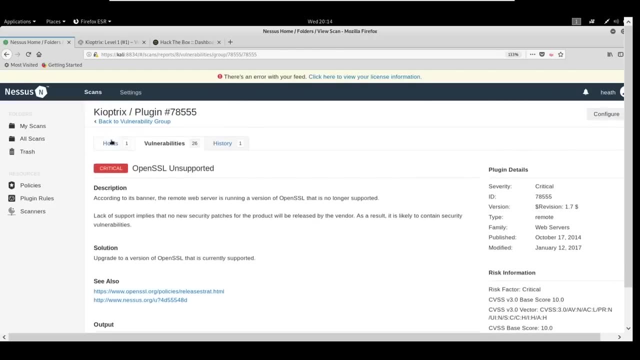 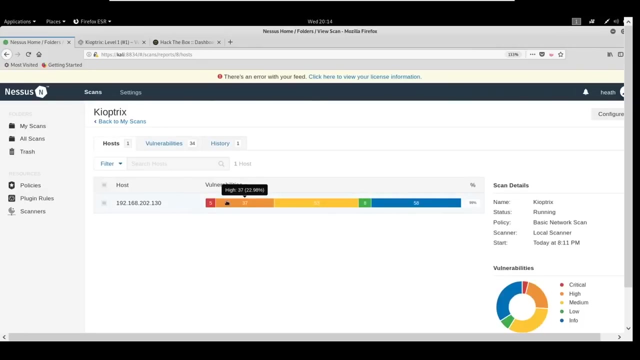 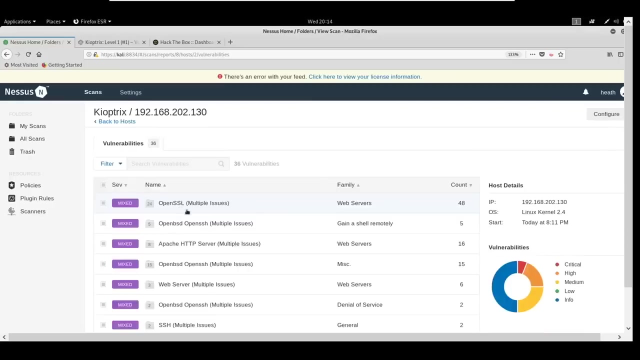 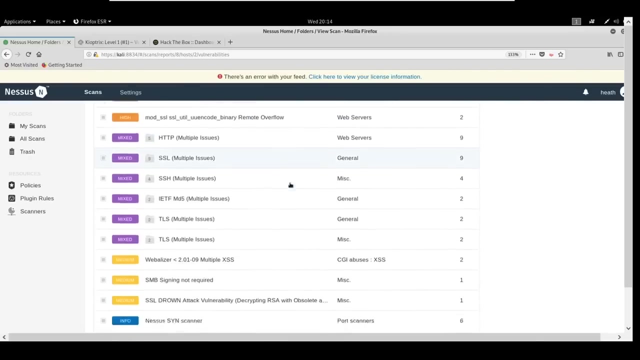 so many things, all the things. there's so much stuff, so let's see if it's done scanning it's still going. we're at 99, though. i also hate the grouping feature i it just came through an update not that long ago and i really don't like it because i like to be able to see uh and sort by the criticals, so i'm not a big fan of. 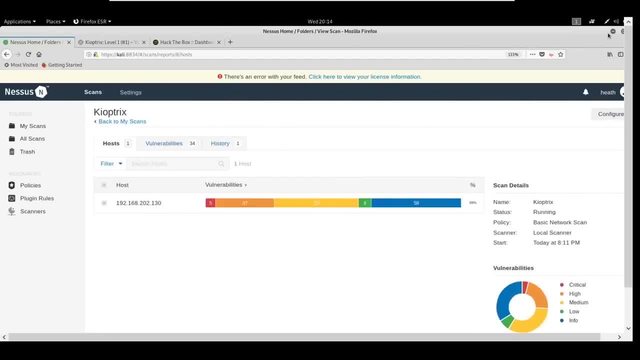 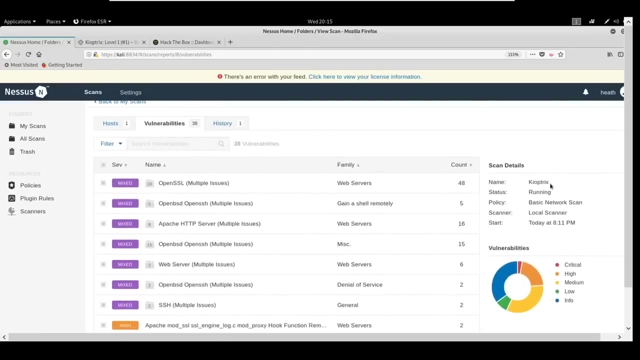 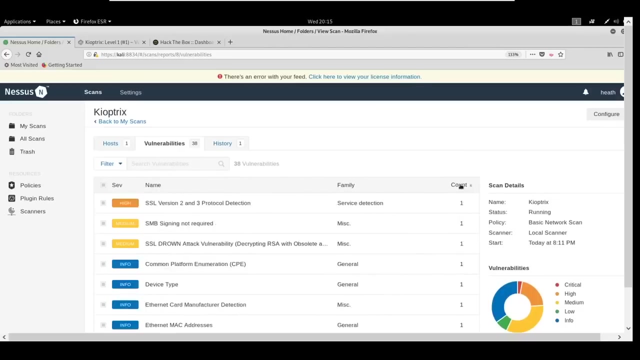 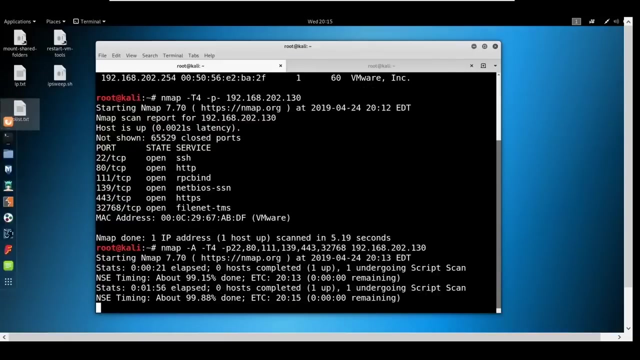 this so I can change it on the interface. oh my man, all right, i'm here. i'm on hosts, click bones. all right, how am i changing this? configure, not configure, click count counts. just sorting, we'll come back to it. check our scan here. so the scanning takes a little bit to get through and this is pretty common. so, like we were talking, 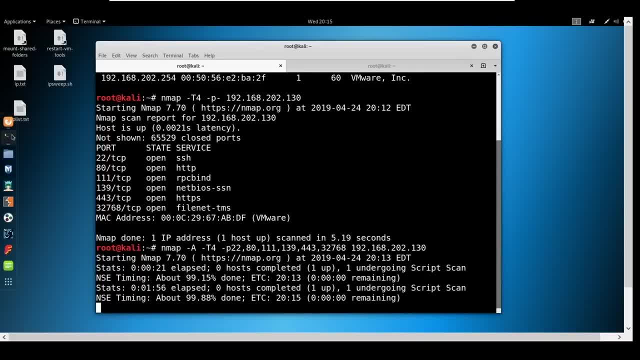 about last week. uh, automating your scans or whatever you give them all that would be really helpful, but we're not going to get through here. the scanning process is going to take us a little不好意思 is always a good idea, so if you know that you have to scan at eight o'clock in the morning, 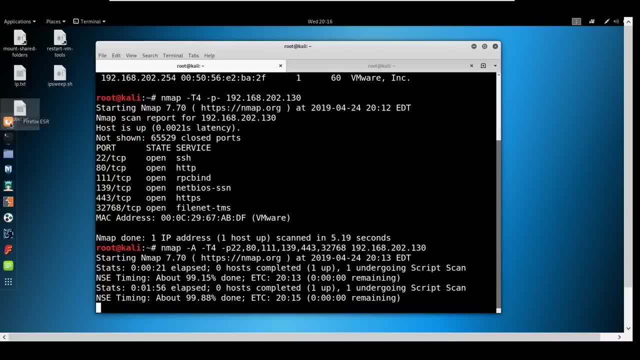 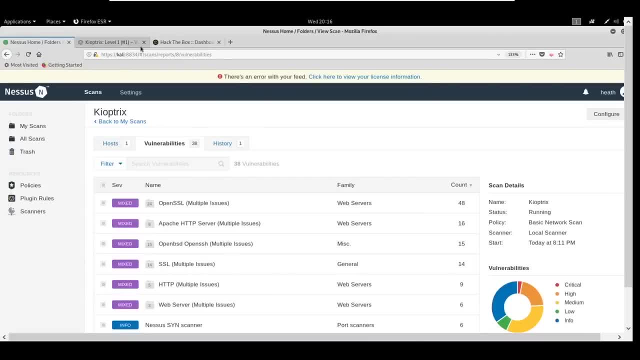 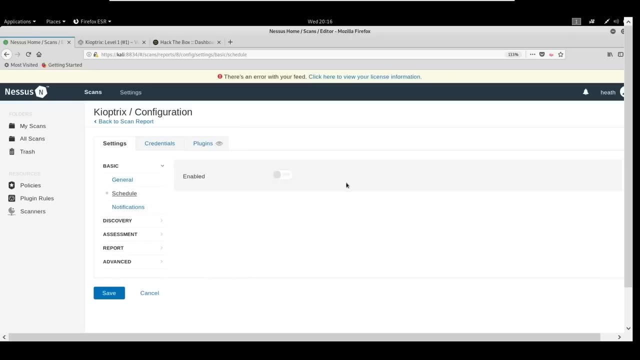 setting up your email to say: hey, client, i'm going to be scanning you. you fire that off eight o'clock in the morning and you also fire your scan off which, if we wanted to configure, there was a schedule in here. we can come in here and enable that schedule and tell it exactly when. 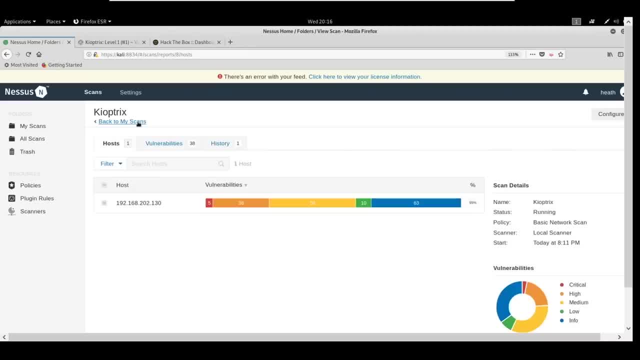 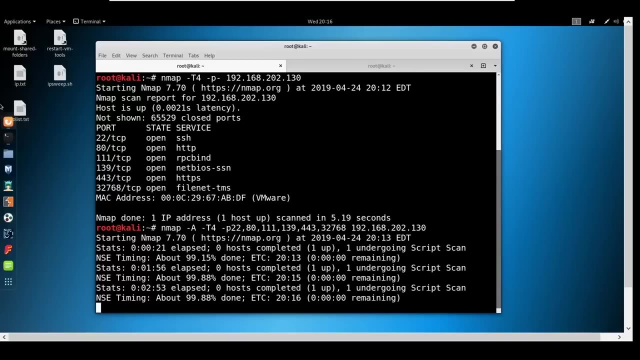 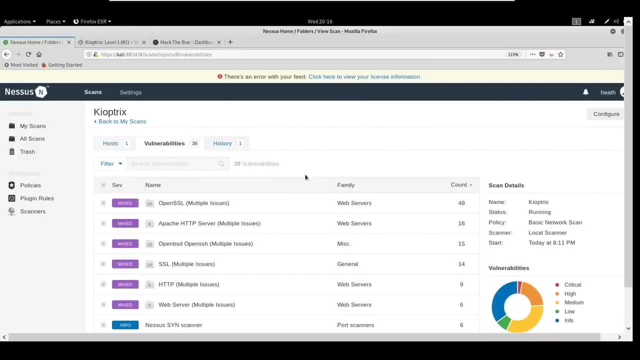 to start and it would do it on time for us. so any sort of automation that you can do with this to save time is definitely helpful and we can start looking through some of the things. while we're waiting, we're still picking up a bunch of vulnerabilities. 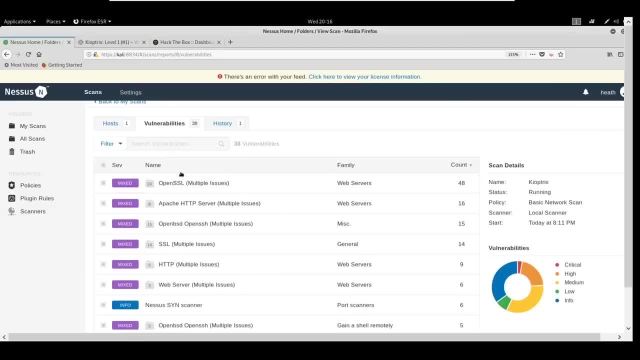 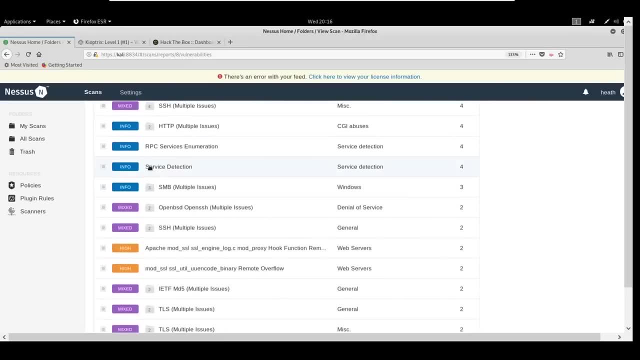 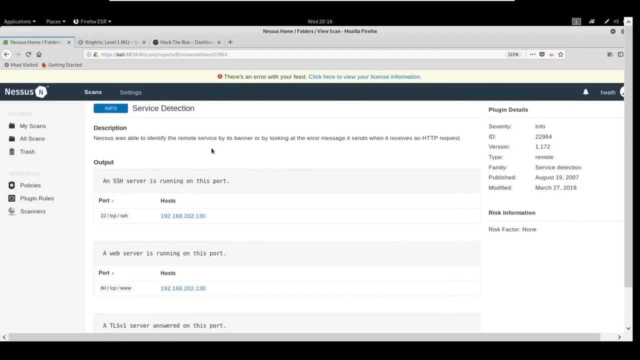 we've got open ssl issues. we've got apache http issues, look like there's going to be a web server. so if you come down and you look for service detection, this is one of the more important things to look at. so it tells us what kind of services it found. so it found. 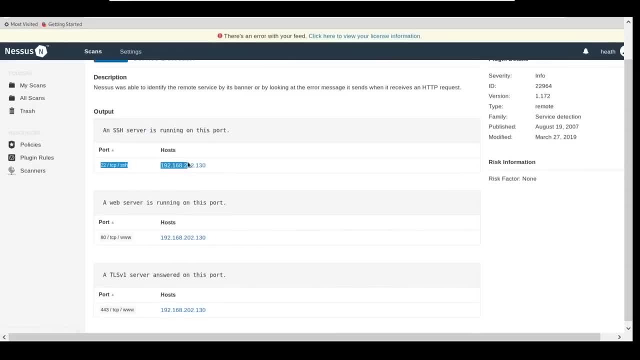 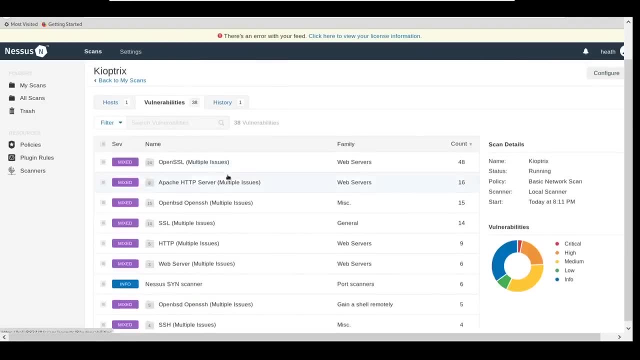 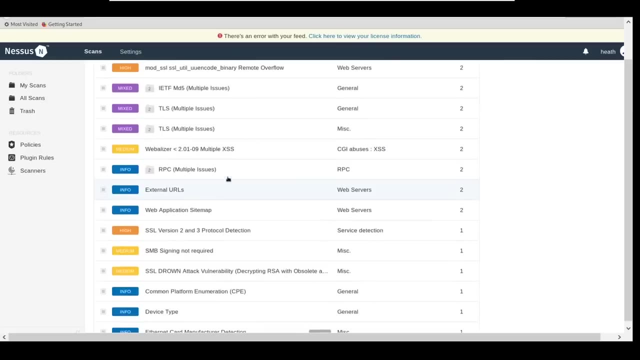 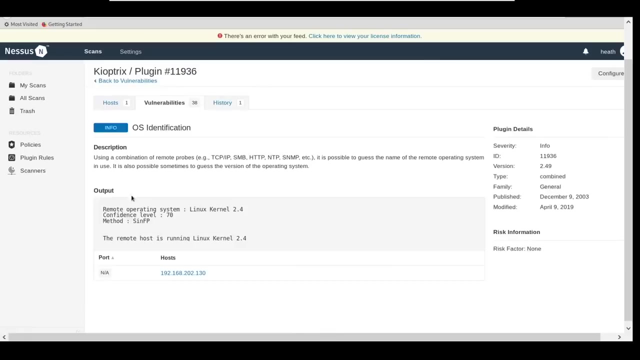 it found a ssh server. it found a web server and found another web server running on 443. it did note that it found smb as well and i'm looking to see if there's anything else. so it provides you all kinds of information, like it says, os identification. 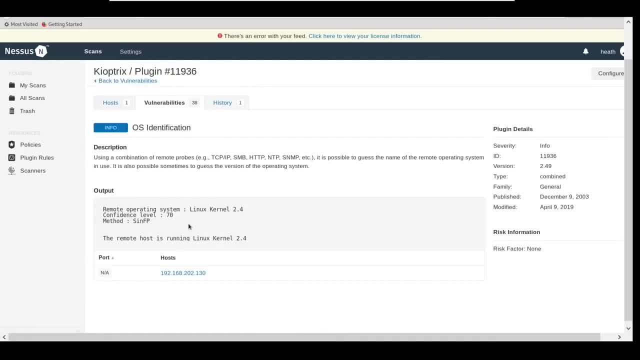 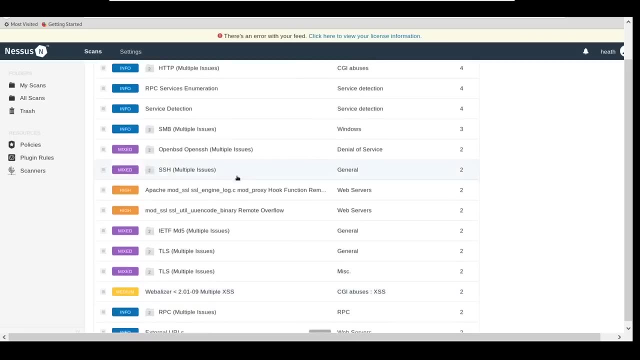 it's going to try to identify the type of os that's running. it says linux kernel 2.4. that may or may not be correct. a lot of times that's a false positive, and before we get into that, let's take a look at some of the things that we're going to be looking at. 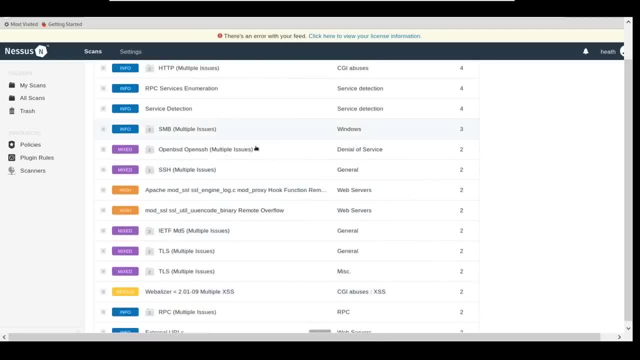 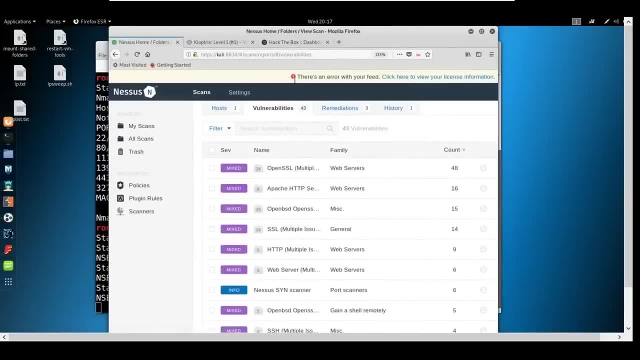 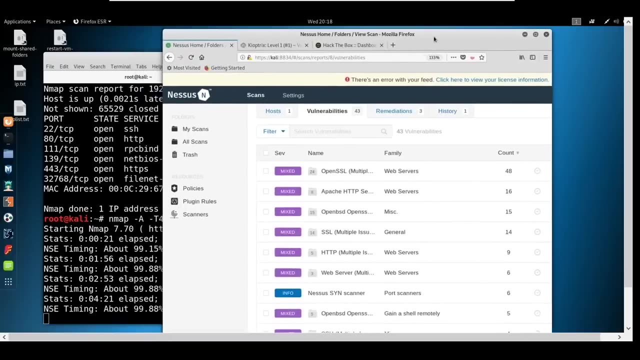 before we dive into this, there's a mod, ssl remote over or, uh yeah, buffer overflow. here i want to get to the nmap before we dive too deep into the nessus, but the nmap is taking its sweet time. so, okay, we do know that there is a, we know that there is a web server out there and, of course, 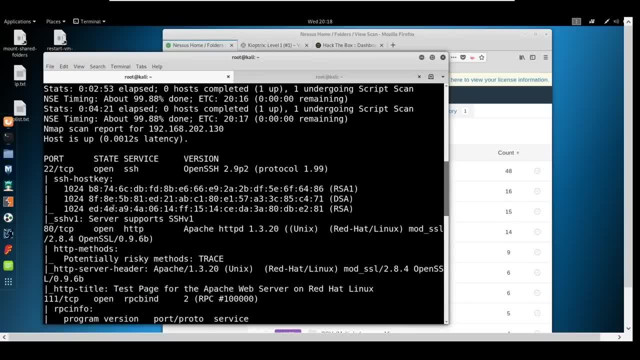 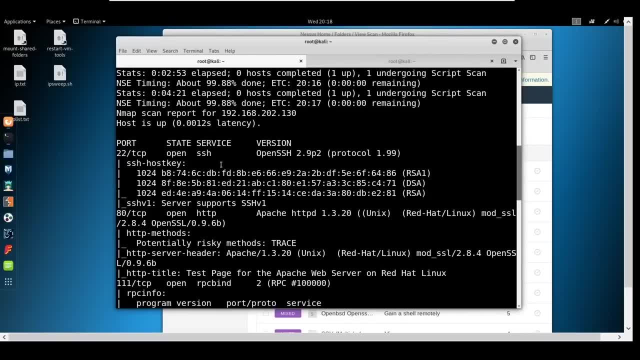 as soon as i'm getting ready to to move on, it just comes through. okay, let's take a look at the scan. so we've got port 22 open. that's ssh, and it gives us a little bit of information here on the version. we've got open ssh 2.9 p2. we've got a web server sitting on port 80. it also gives us a version of. 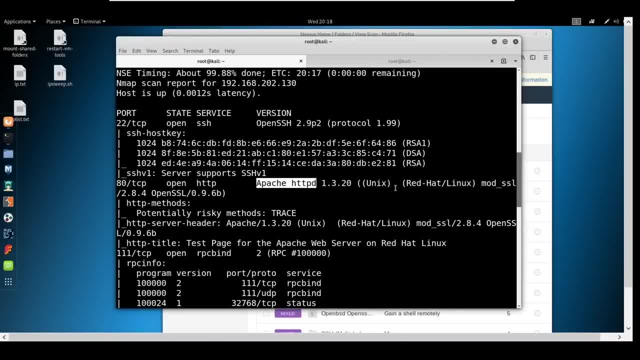 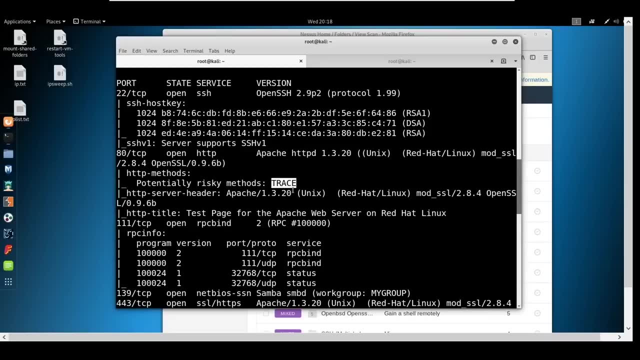 apache. http d 1.3.20 also says that it's running red hat linux mod. ssl 2.8.4. open. ssl 0.9.6b identifies a trace method and identifies the server, which it already did once, but it's got that as well. 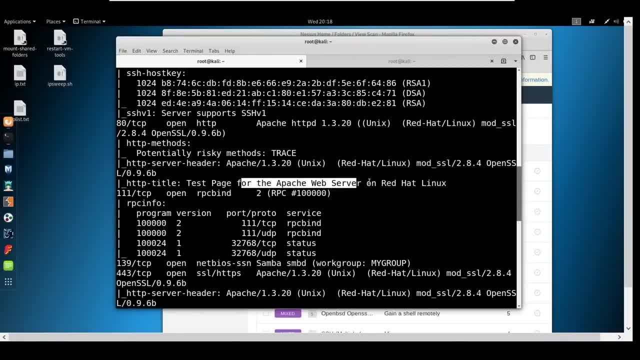 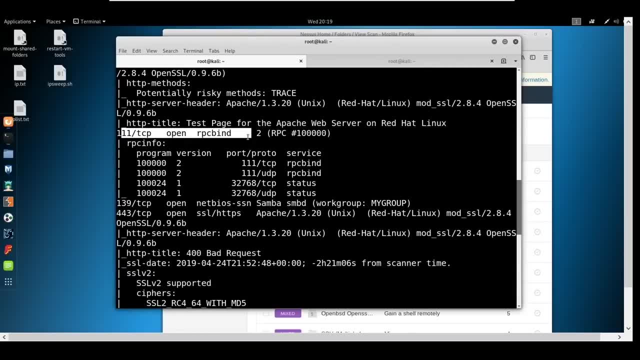 and it says: test page for apache web server on red hat linux. okay, uh, 111. here rpc bind. typically we see rpc bind when we have- uh, we have 139. we have sambar smb open, so that is a common pairing here. so we've got 139 open. 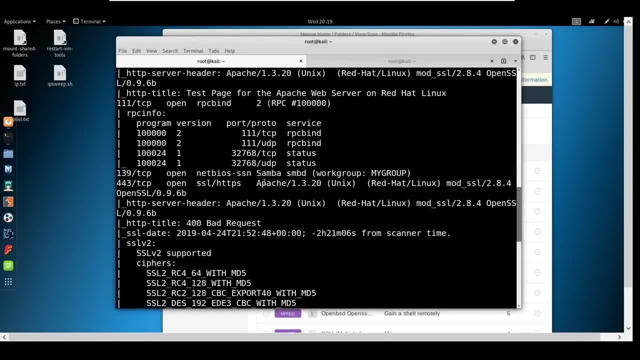 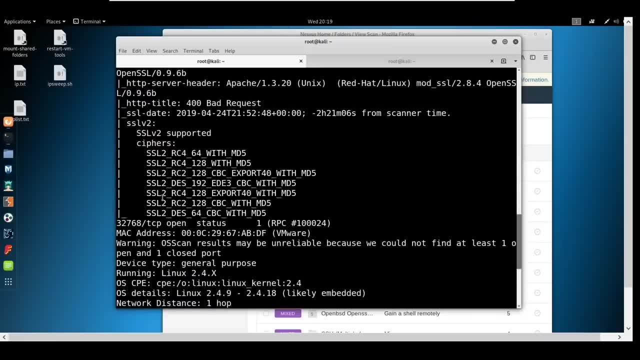 we've got smb 443. looks like it's the exact same thing as the port 80. uh, we'll have to give it a look and see exactly what we see. and then we've got this 32768. uh, also looks like it's an rpc bind. 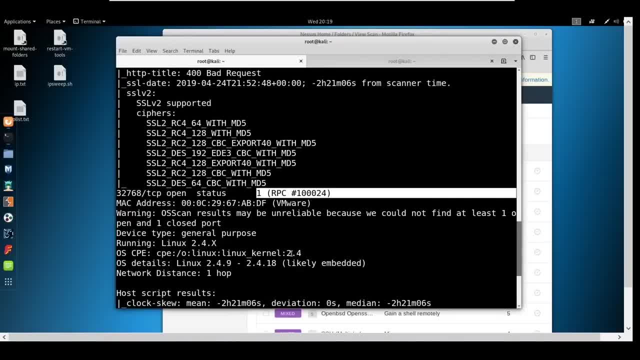 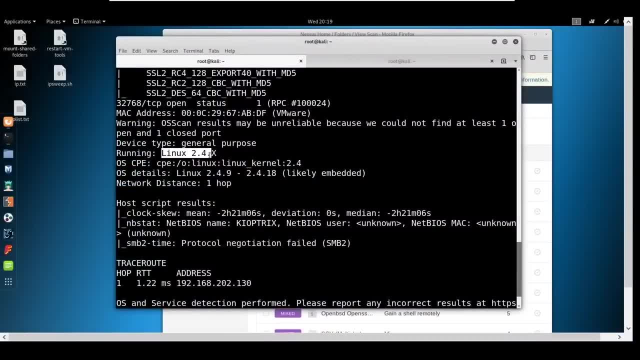 of some sort, because you can see the rpc here. uh, so we scroll down. it gives the best guess of what kind of linux it is: linux 2.4. this is not all the way through, so we're going to scroll down and see what kind of linux it is. 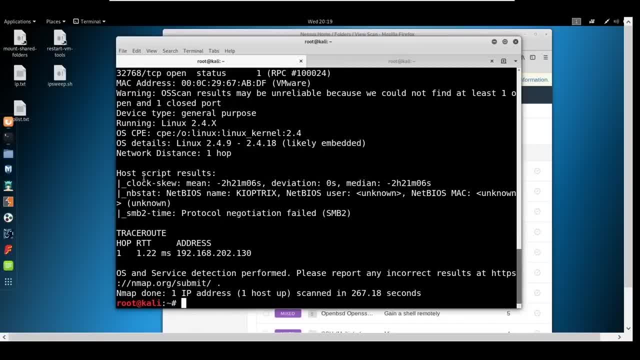 this is not all the way through. so we scroll down and see what kind of linux it is: linux 2.4. this is not all the way through, always accurate. this is just its best attempt. uh, it comes down here and it does smb. it looks at it, tries to identify what type of smb it is. 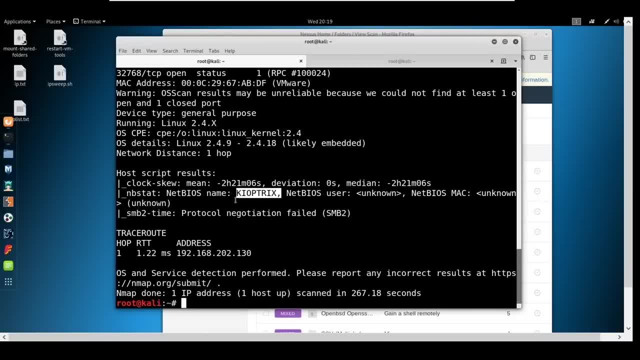 it doesn't really identify um. it does identify a host name of keyoptrics- okay. it doesn't know a user, um doesn't tell us really anything about, uh, anything. so this is where having multiple scanners comes into play, because there's already things about this smb that i noticed. 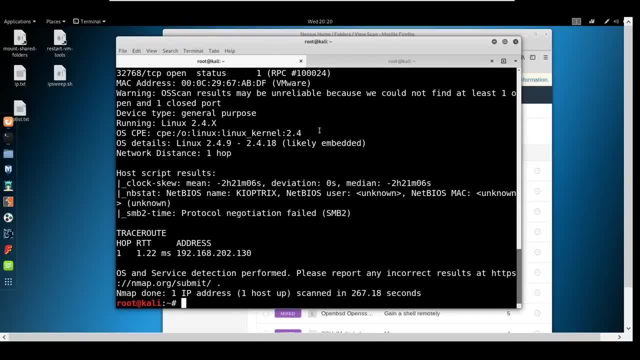 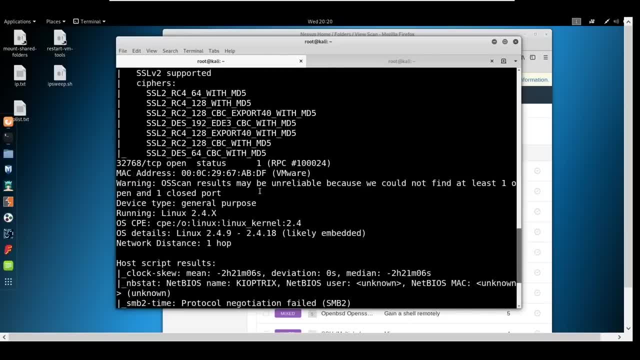 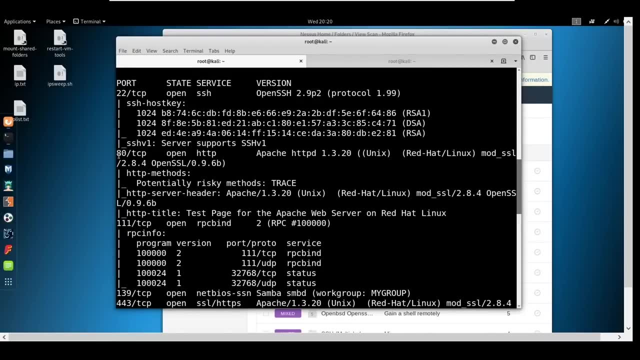 that in the nesa scan that's not showing up in this gap. so as a pen tester, i'm going to be looking for the low hanging fruit if this was on the external web server. the first thing i want to be looking for is port 80. i want to see what they're running on port 80 or port 443. 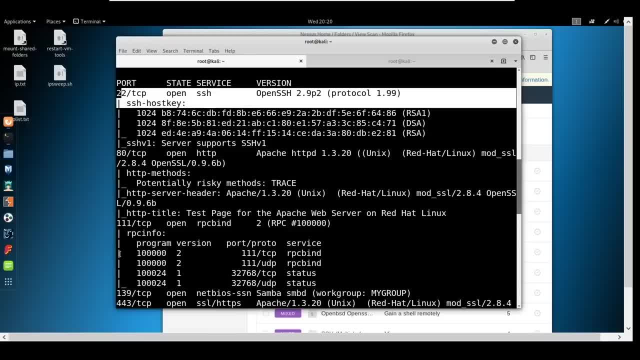 i also want to know why they have ssh and why they have 139 open. now, this is on the internal. okay, 139 opens not as big of a deal. we know why: because they're likely using a file share and ssh. okay, they may remotely administer the machine in some way or another. so these would 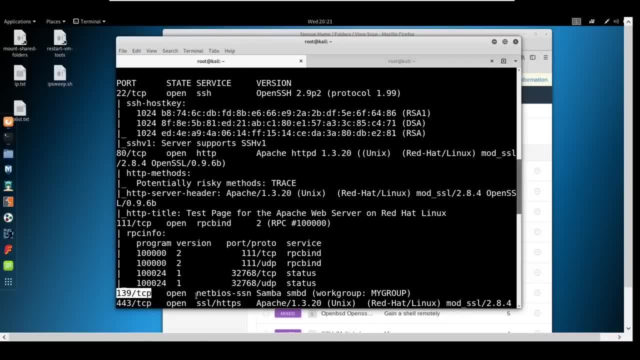 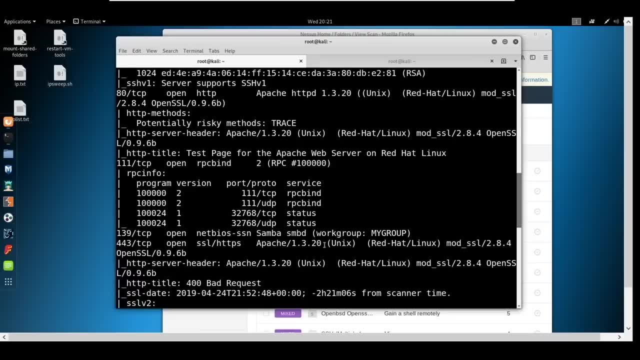 be bigger concerns if this were on an external network. same thing with if you see something like rdp on the external network. that's something that you would be: uh okay, why is that there? you know, uh, internally again, not as big of a deal. there's vulnerabilities that we can. 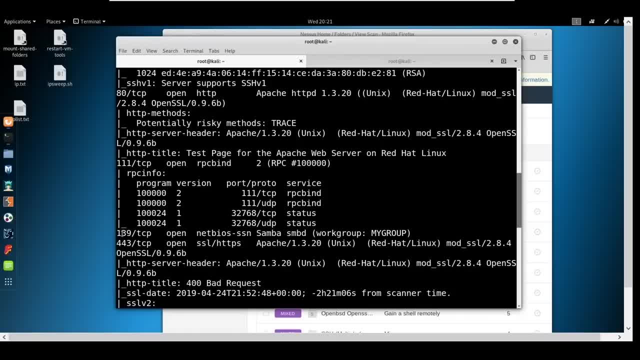 exploit and we're going to get into that when we get into internal exploitation, when it comes to 139, but we're not going to get ahead of ourselves so low hanging fruit in the order that i would look at this. i would probably look at this at either port 80- first 443 is included in that- or 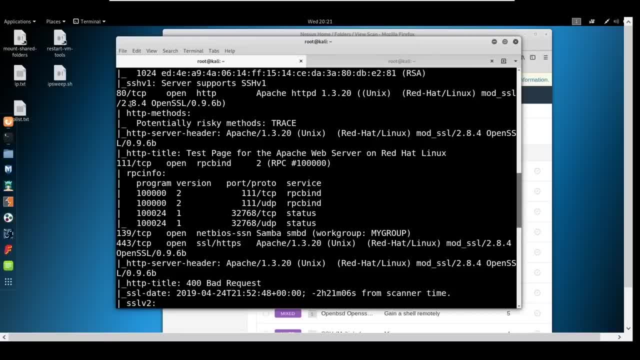 139 as well, mainly because there's a ton of smb vulnerabilities out there that lead to remote code execution. there is also a ton of vulnerabilities out there that are web related. so if we're doing a network pen test, we need to make sure that when we go out to these websites- and we talked about this last week- that we're not doing a web. 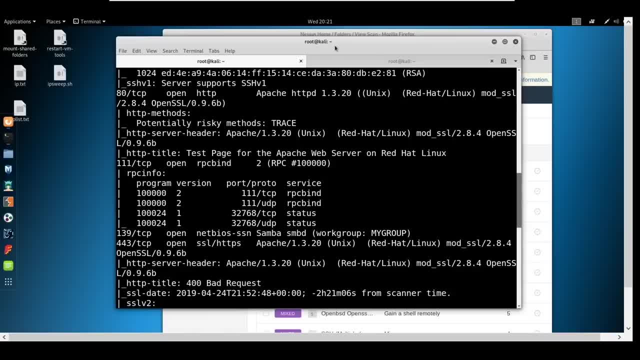 app assessment. we're not going to be looking around for anything and everything. we're looking for some sort of direct win. if there's a login page, we might try to brute force the login page. if there is a login page, we might try to do sql injection. but we're not looking for like 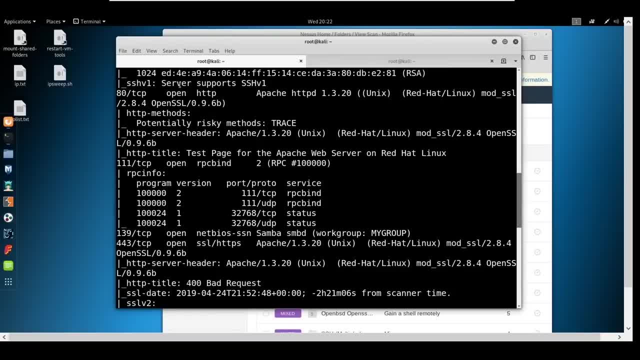 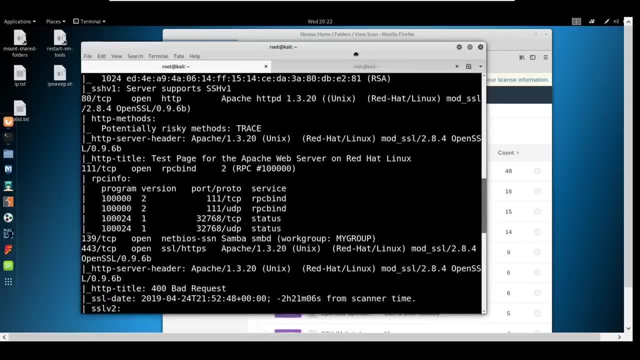 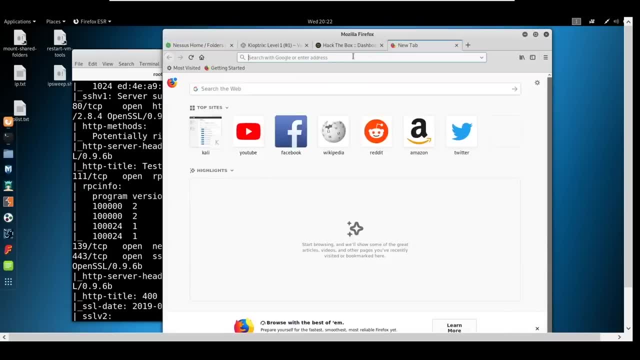 cross-site scripting or we're not going to report back on certain headers being missing and things like that, but let's go and just navigate to the page. so our first step of enumeration is: we're just going to go take a peek at what the page looks like. so again, we are sitting at. 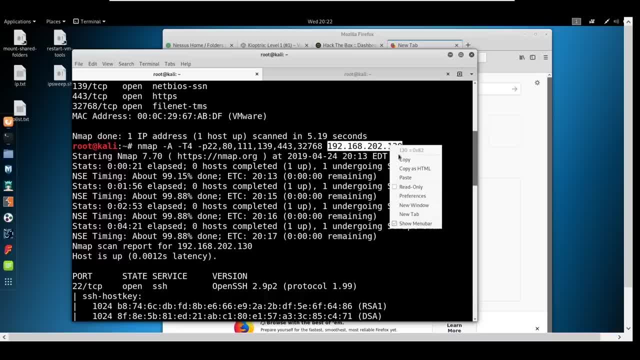 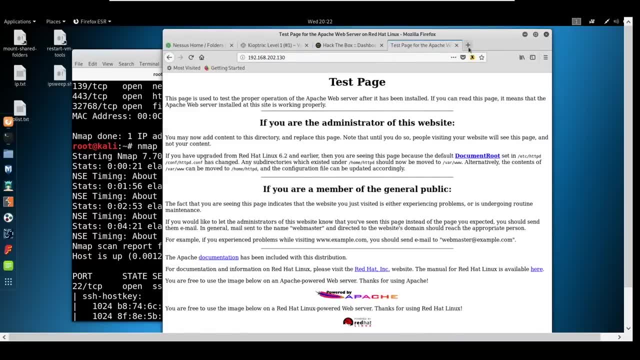 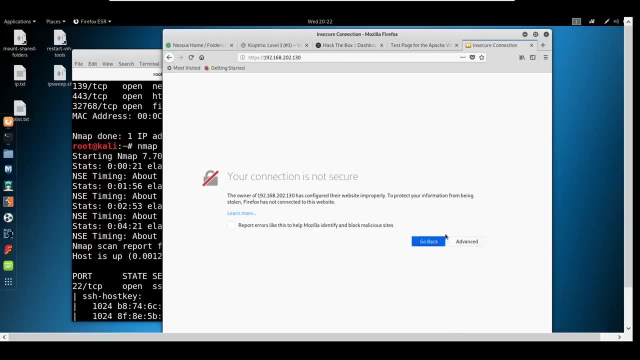 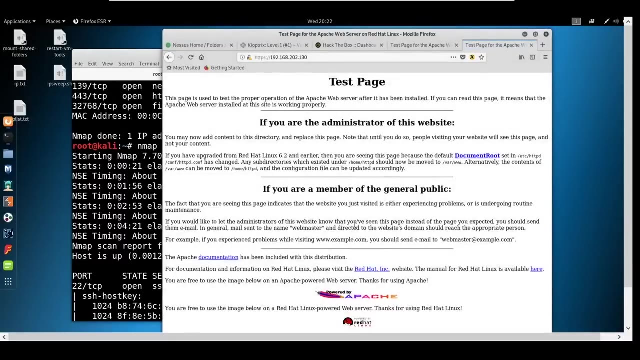 192.168.202.130. i'm just going to copy that. okay, apache test page. i just want to see what it looks like on the https side. just say advance, add the exception. you can confirm the exceptions. also a test page. okay, so for me this is finding number one. you've got a default test page on out in the open. 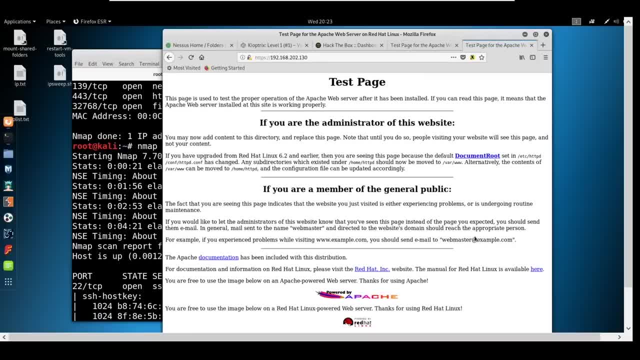 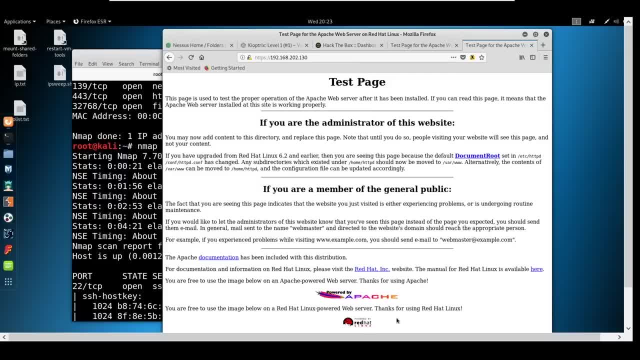 by apache. we've got that. it's powered by red hat. okay, so now we're giving out server information of what type of framework we're running, what type of operating system we're probably running on on top of that. it just signals that this client here might have poor hygiene. 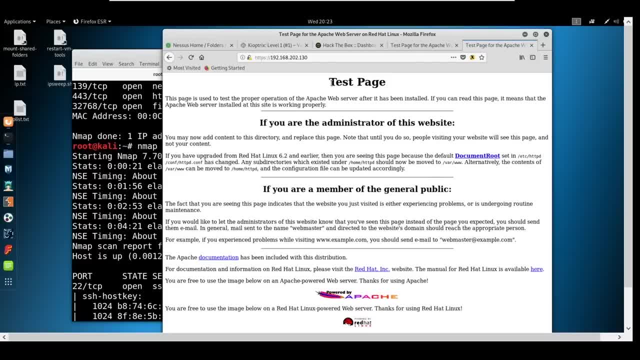 if they're running a default test page out on the on the web, why are they doing that? is it because they forgot to take it offline? did they just leave it up? or are they running a server somewhere on this ip address but they forgot to take down the desk page? you know, i've seen a lot. 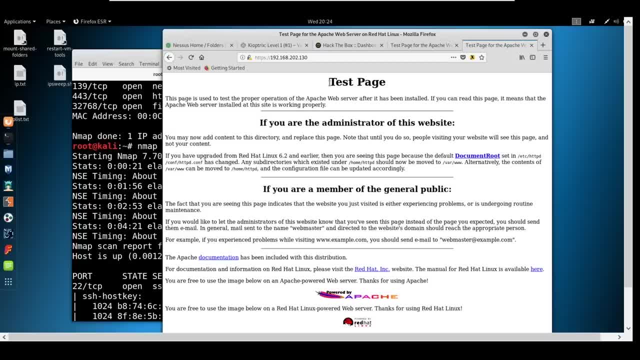 of misconfigurations. so what you're looking at here is you're saying: okay, if you're an attacker, from the attacker point of view, you say: i see a test page, that's the test page, that's the test page. that's poor hygiene if they're leaving this sort of misconfiguration just out in the open. 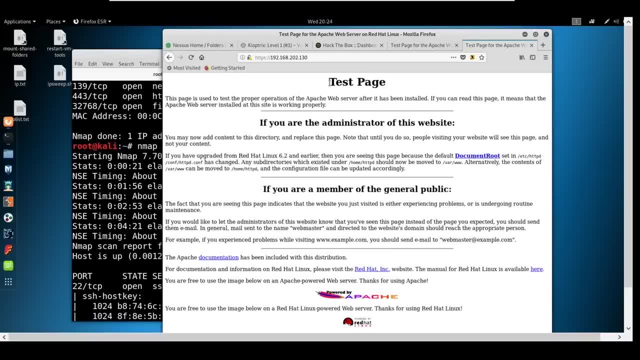 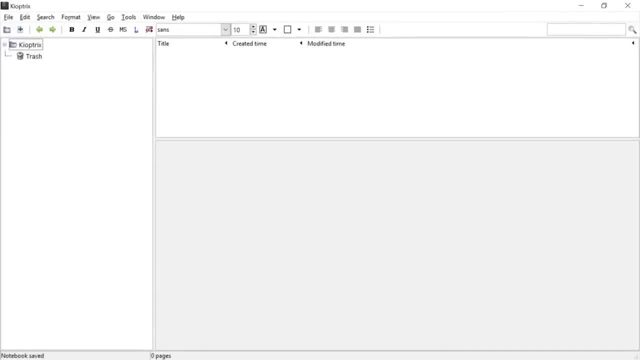 what other sort of misconfigurations are out there. so we're going to go ahead and notate this, this issue. so what we'll do is we'll come into here and i'll make a child page and we'll just call this, uh, vulnerabilities, and then we'll make a new child page. 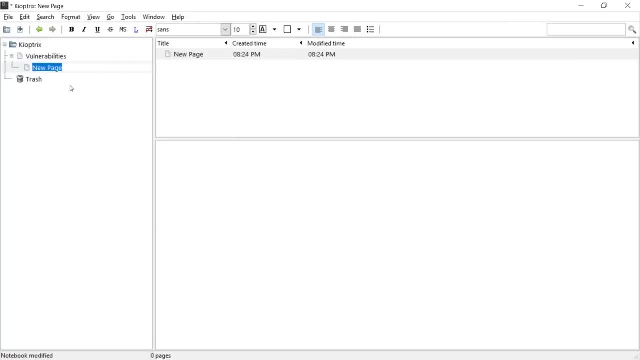 and we'll say: and then we'll make a new child page and we'll say default web page and we'll just call this low. so we want to identify a couple things we want to identify. if we're doing multiple ip addresses, we'll identify um, we'll identify which ip address it's tied to like. if we're 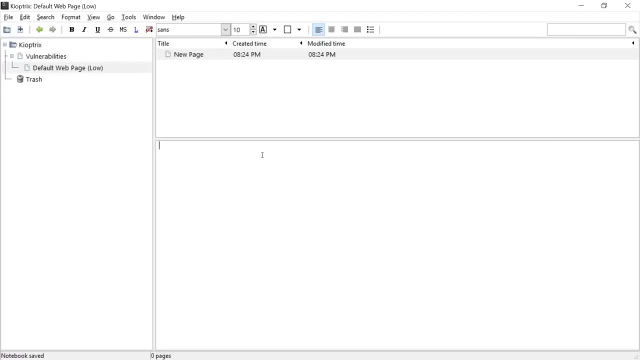 scanning a network, a subnet of, like a slash, 24 um we'll. we'll use, uh, the specific ip address we found it on. so in this case- and i keep forgetting it so i'm not typing it out- 192 sang ones six six eight two zero two one thirty. 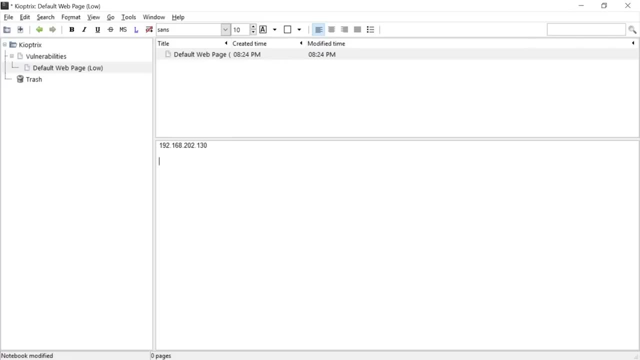 so we'll notate the ip address. uh, we might put some sort of notes in here for ourselves if it's uh, not self-explanatory. but this one is pretty self-explanatory. and somebody asked what the uh, what the notetaking application is. this is: keep note. 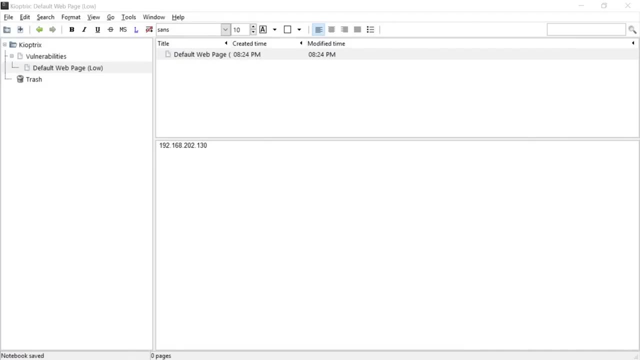 so it runs on mac and on windows, i believe, or it runs on phone and im infotainment. it appears to be a good app right now and i've located it here in our. based on of the print app up here kind of says it's 1946: 19 yağels uh the white 한번어. 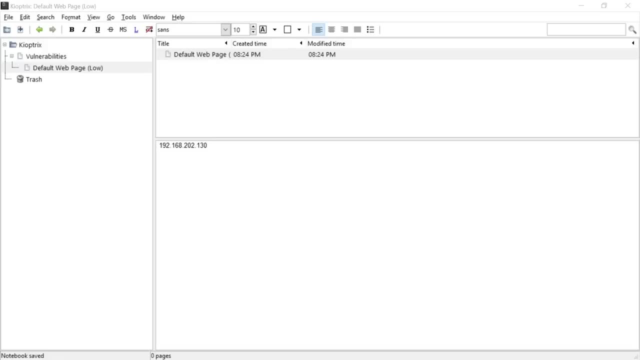 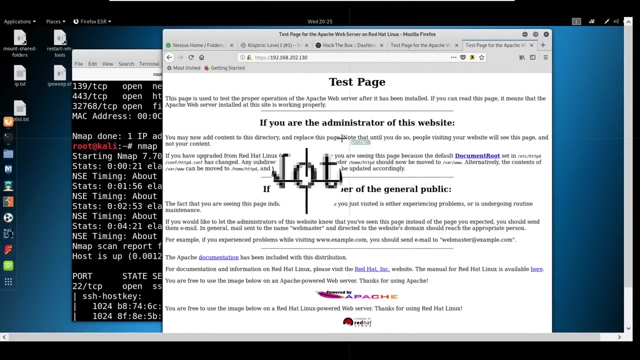 it runs on Linux and Windows. I don't remember which, but it definitely runs on Windows. Okay, so we're also going to use our screenshot tool, which is Greenshot. Let's minimize this. I'm going to take a screenshot here of the test page. What I like to do is I like to get in here. 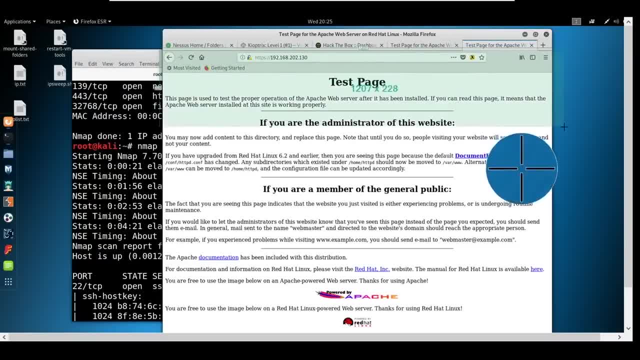 and I like to make sure the IP address is in there. It doesn't have to be the whole test page, It could just be something like this, and this might even be too long, to be honest with you. You might need to shrink it down just for reporting measures. 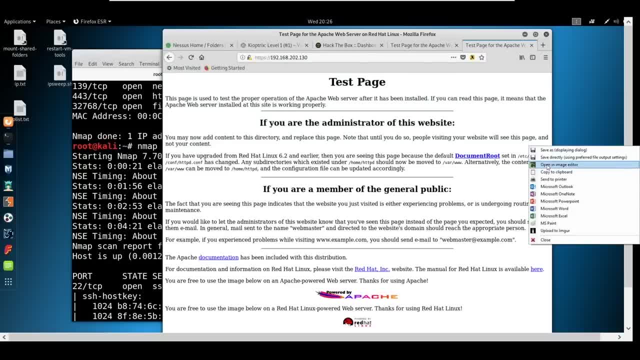 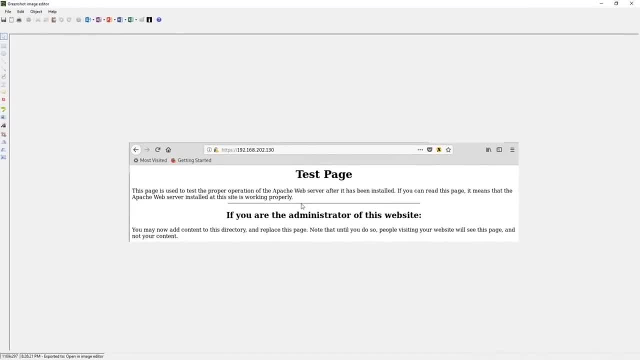 but come in here You say open an image editor, and I'm going to drag this over you so you guys can see it. I like to make it pretty, so I like to come in here and I like to add a border. 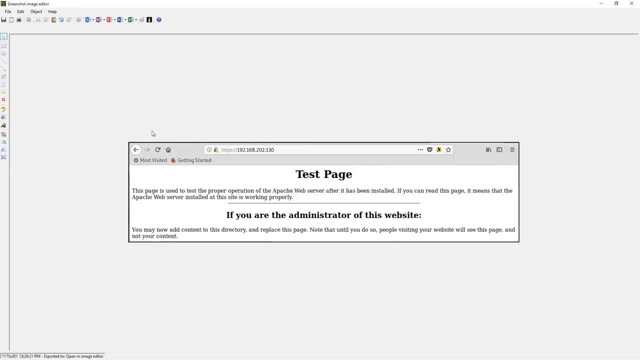 so it gives it a nice little border in here and some other cool little things. I know we've covered note-taking before, but if I want to highlight something like, say, okay, test page, I want to highlight that it's a test. 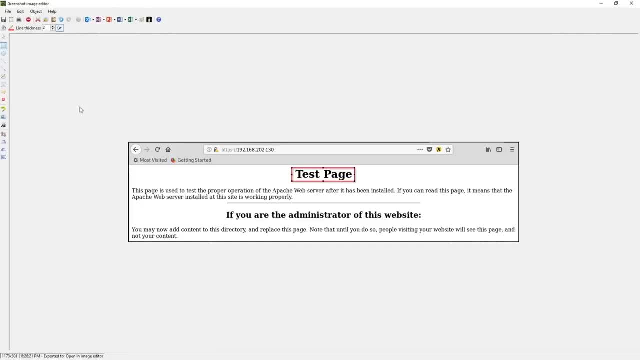 page. I'll do that. If I need to highlight the IP address, I can do that. There's obfuscation in here as well. If I need to blur something out, we can also do that. I'll just hit the copy button over. 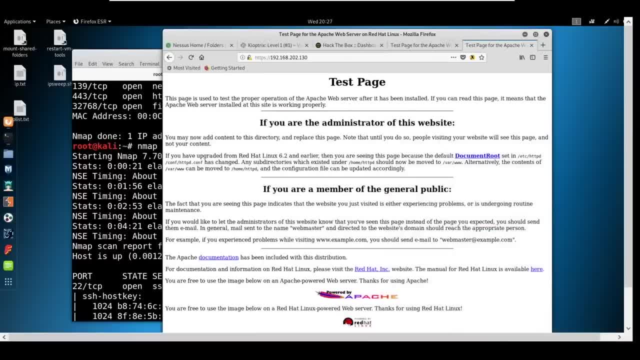 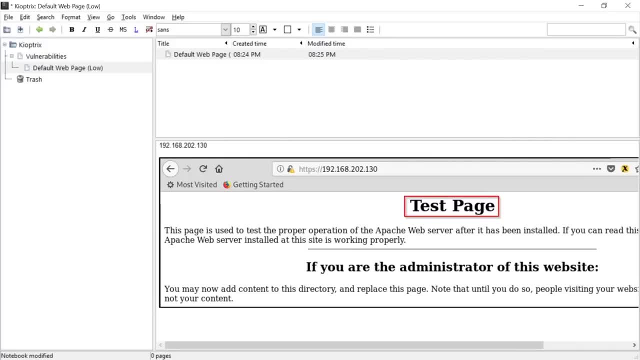 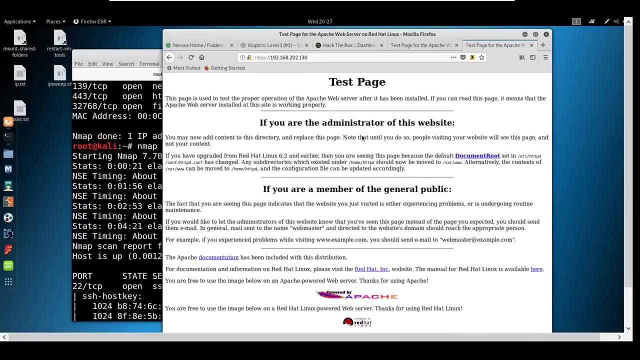 here, copy the image to the clipboard, come back into our note-taking application and I'll just paste it into here. All right, so that is our very first finding. We see here that we have our test page. I mean, if it were a real website, we could view the source and see if there's anything in the 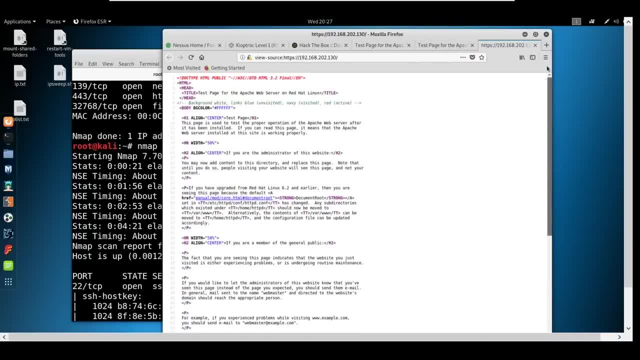 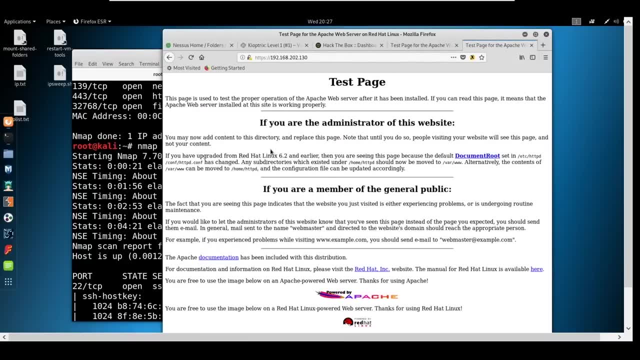 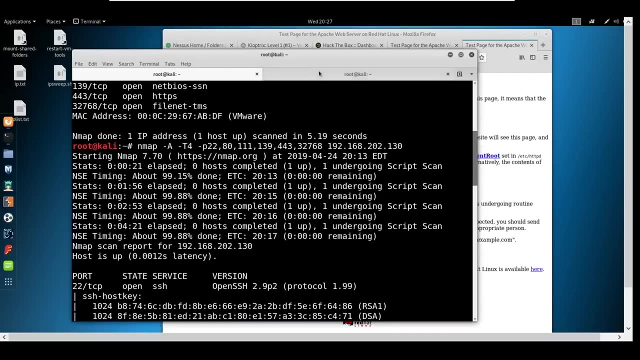 comments or something off of the source code, but since it's a test page, pretty much nothing going on here. When we have port 80, we've got something here. We've got something here. We've got something that we can use, some tools that we can use built into Kali that allow us to enumerate. 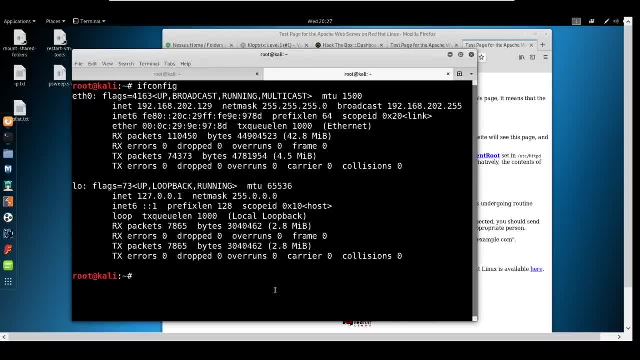 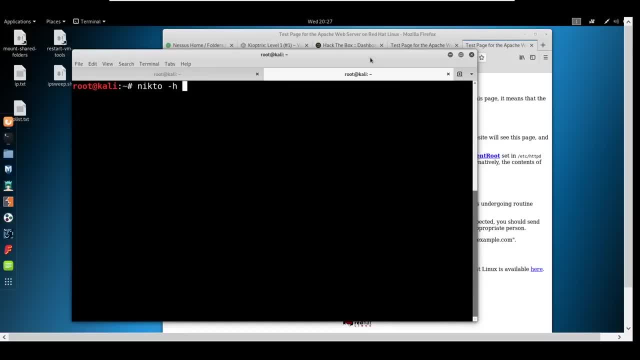 We talked about this last week. Number one is Nikto. Let me clear the screen. We're going to run Nikto on this host. You do a Nikto-H for host and then you just type in 192.168.202.130. 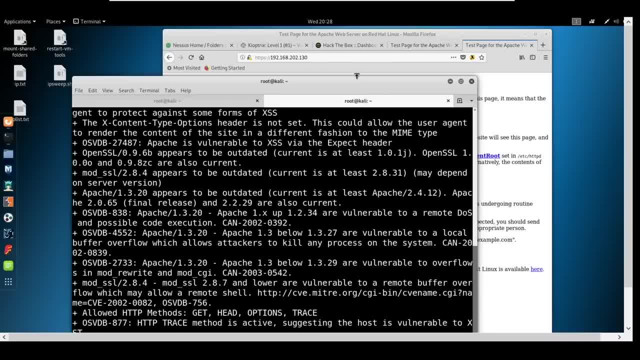 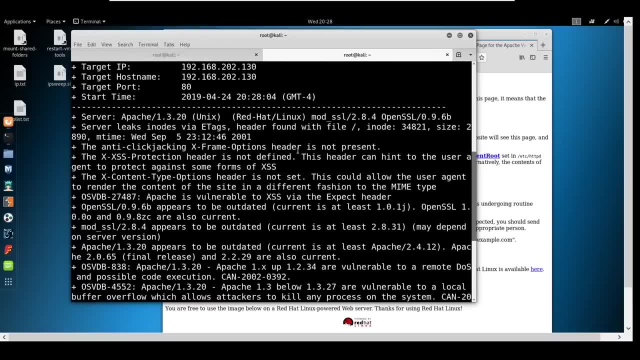 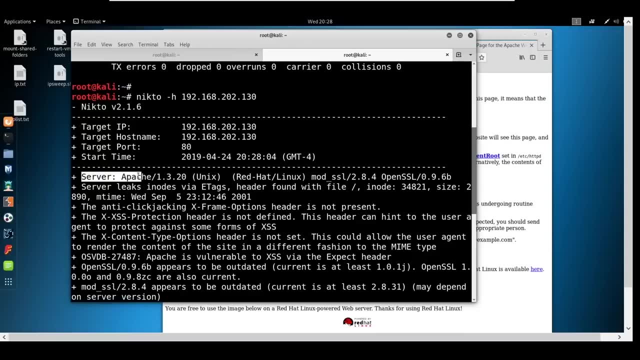 and hit enter. You're going to see it's just flying. It's flying through already with all sorts of information. So again, if we look at Nikto, it's pulling a server header from a response header here and it's pulling Apache 1.3.20.. That is going to be a finding. Usually I'll go into Burp Suite. 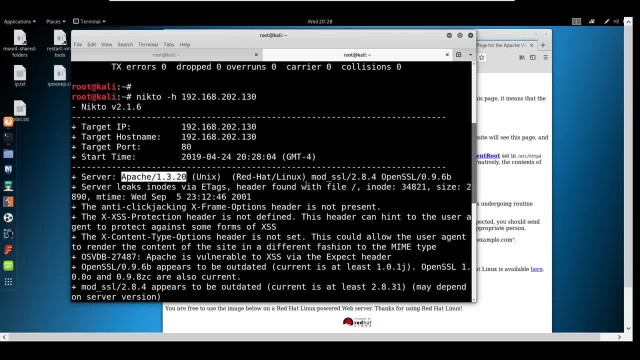 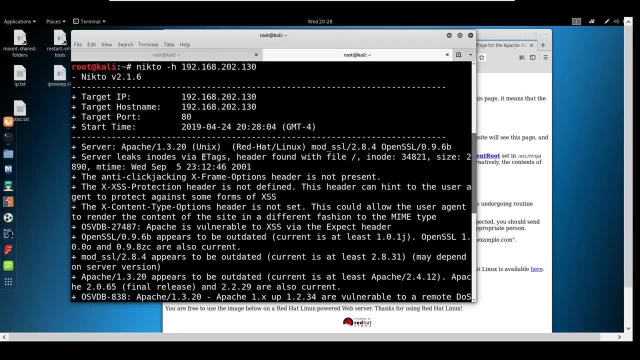 and take a screenshot like a prettier screenshot. I probably won't take it from this. here You're seeing the mod SSL again. It's leaking e-tags. That's not something I would typically put in an external finding. That's just kind of nitpicky. And the same goes with these These. 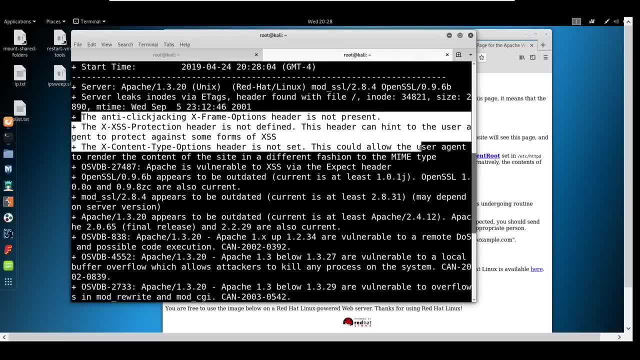 are findings for a web app assessment, but they're not findings for an external assessment, unless for some reason we have found absolutely nothing and we need to put something on the report. But typically we'll find a little bit of information, and especially tonight. 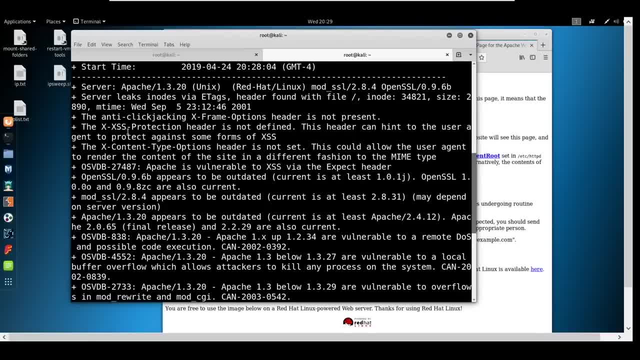 we're going to find a lot of information. So we look at this and you've got these headers that are missing right: The anti-click jacking, the cross-site scripting, protection, the content type. So we're not going to worry too much about. 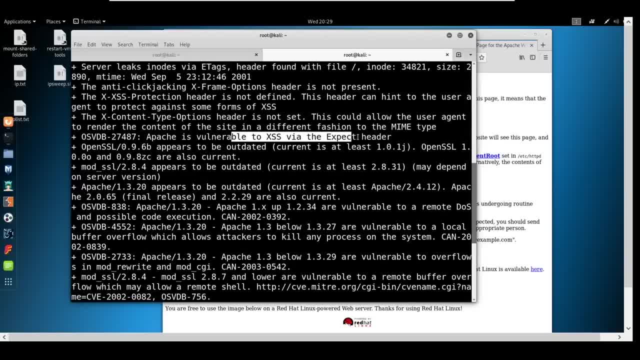 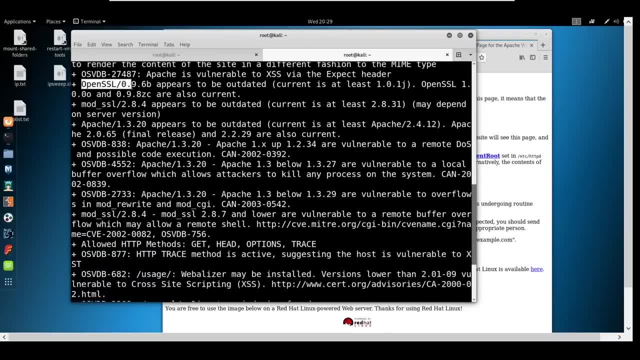 those. We're not going to worry too much about this cross-site scripting. Again, this is not a web app assessment, but we do worry about SSL. This open SSL appears to be vulnerable. This mod SSL appears to be vulnerable: Apache 1.3.20.. That is going to be a finding, So we're not going to 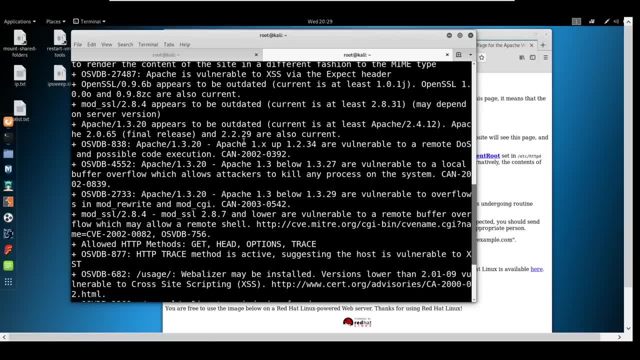 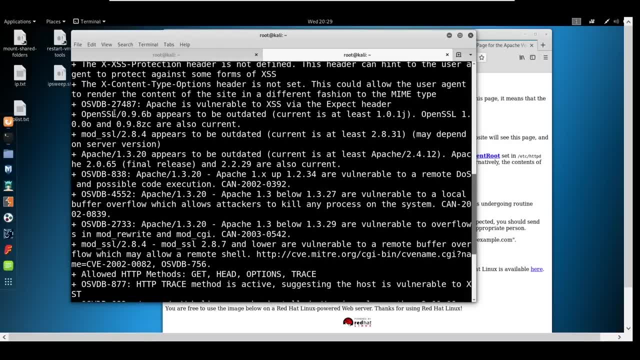 zero. It appears to be vulnerable and it's going through and kind of doing a little vulnerability scan for us. So these are all things that we're going to want to look into and do some research on to see what the vulnerabilities are that exist and how we can look those up. What can we use to? 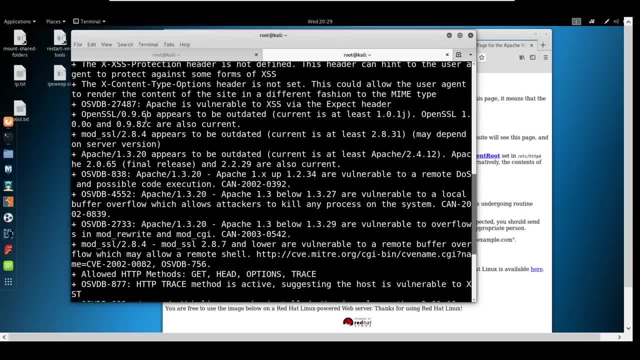 our advantage. What kind of vulnerabilities are they? Are they denial of service vulnerabilities? Because, like, say this, remote denial of service, Yeah, that's something we're going to report, but that's not going to be something that we're going to be able to act upon, because most of the 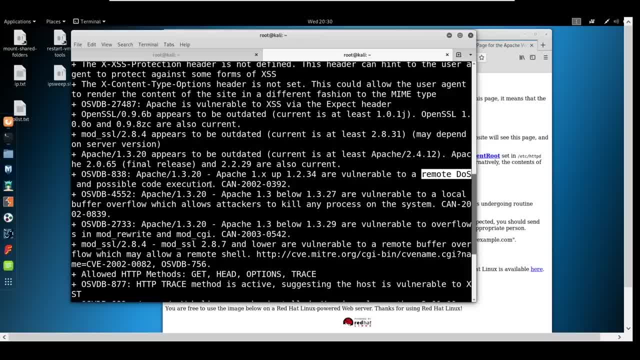 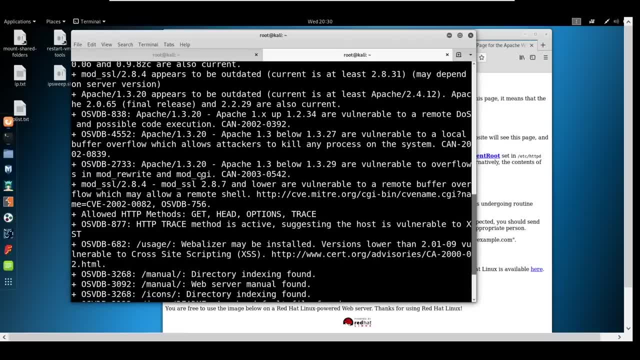 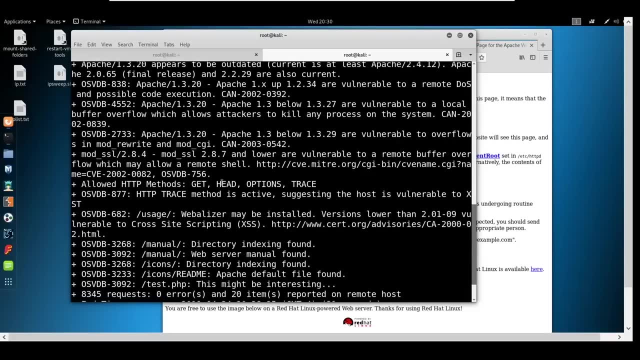 time. denial of service is out of scope when we're doing these sorts of assessments, But it's definitely something we would notate saying it's vulnerable, So we'll get back to that in a little bit. We'll scroll through the rest of this. We see the allowed HTTP methods and get head options. 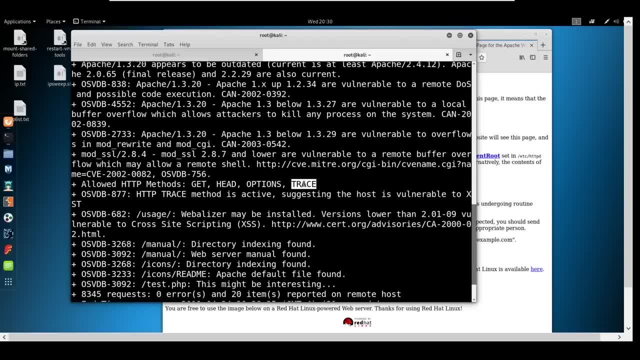 Those are all fine, Trace is. it's a little risky to have trace on, but only if we were able to find some sort of cross-site scripting. Then trace becomes useful Cross-site tracing. So again, this is nitpicky on an external assessment If we were doing a web. 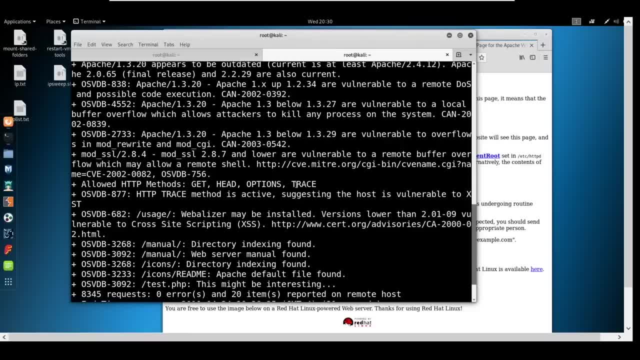 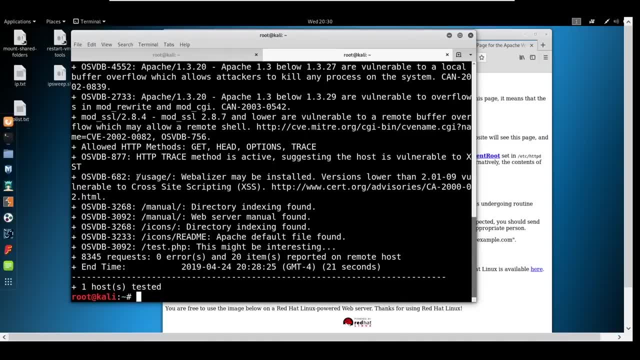 app assessment. maybe we'd throw this in there. So we come into here and what else we see? We see that it does a little dir-busting and we've got the usage manual manual. Okay. So it's found some directories for us that maybe we might want to look at, but we're going to do our own. 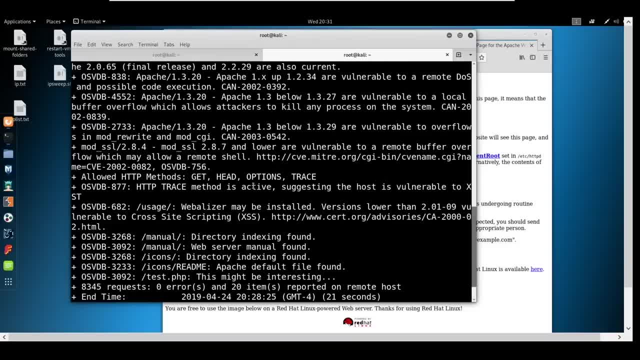 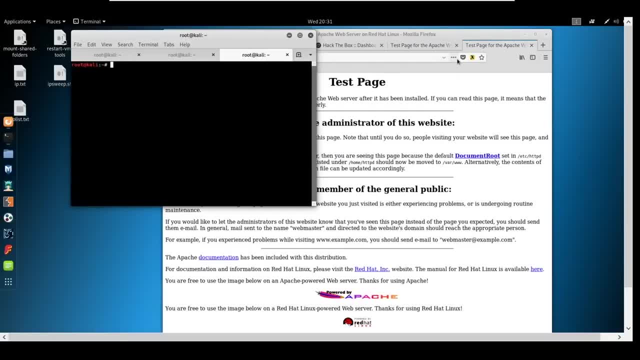 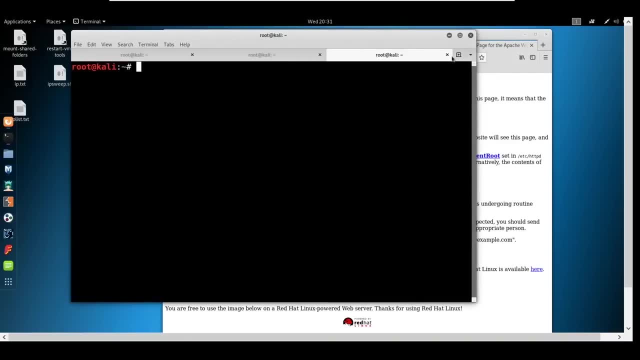 dir-busting here as well. So now we've got a whole list of information that we can go on, And now I'm going to blow this up. Question is: would I normally pipe this out to a text file? So there is a HTML version of. 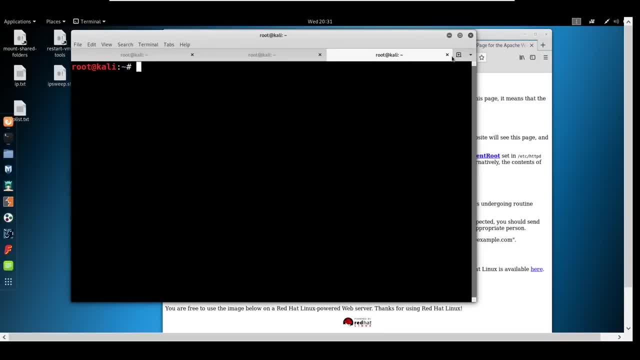 Nikto, that's out there. You can save it out to an HTML and make it way more readable than this. We'd have to look at the options, but that is something that is possible. So yeah, you can make it look cleaner if you're not comfortable reading it in this sort of method. 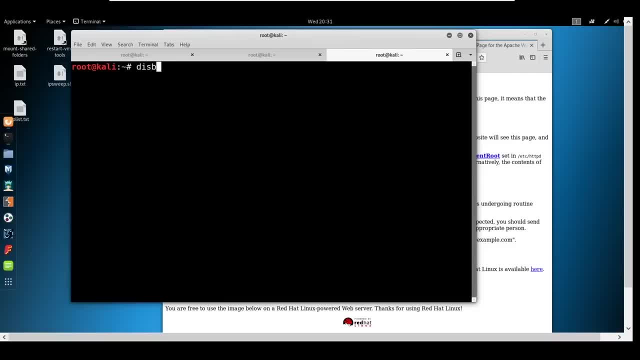 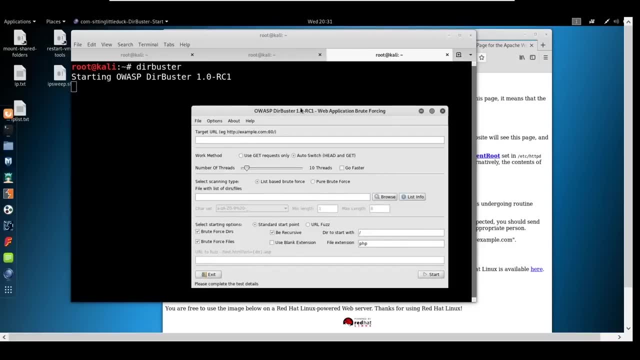 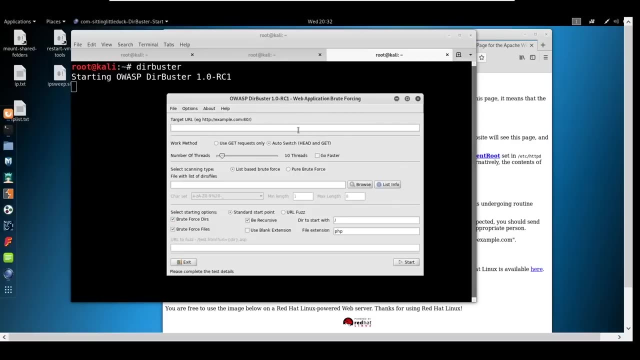 So let's go ahead and run dir-buster. All you do is type in dir-buster like that. Okay, So now it's going to ask us for a few things And all we're doing is we're doing brute-forcing the directories, So we're just looking for any type of file or directory that. 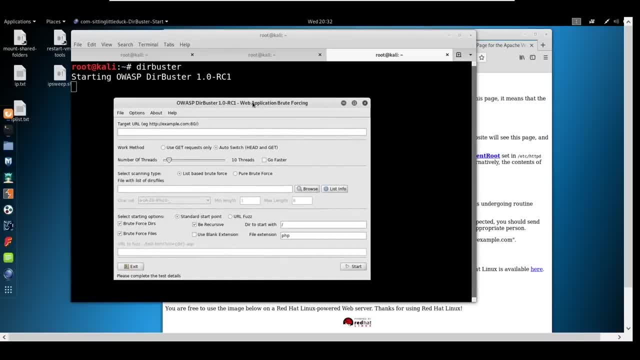 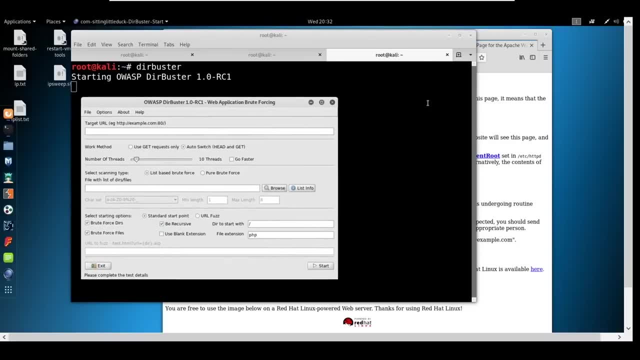 we could use to do that. So we're going to go ahead and do that. So we're going to go ahead and find that we're just not seeing right away. We could also crawl the web page with something like burp suite, like we did last week when we were looking at Tesla, But we're just going to go ahead. 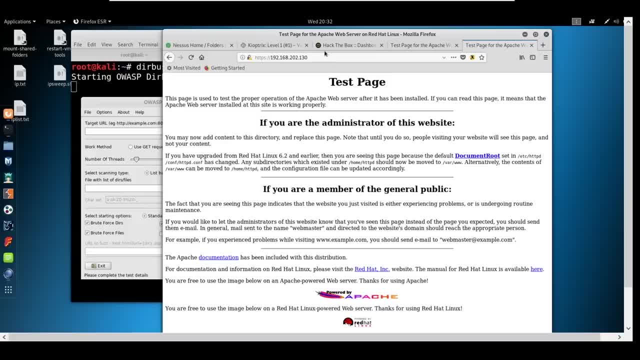 and just look for directories while we wait, especially on a page that's like a test page like this. We want to dig in and see maybe there's a hidden directory, And I have found hidden directories on default web pages before, So, and they had like directories hidden back. 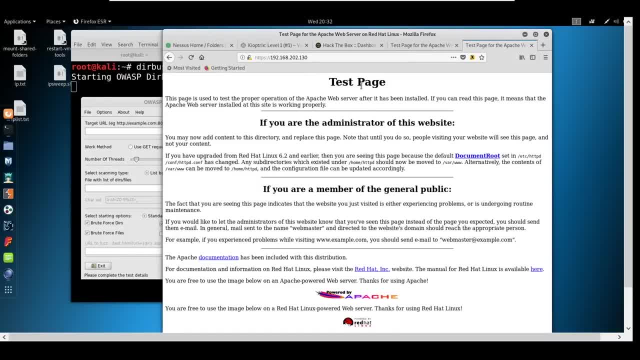 there that were just full of data and information that shouldn't have been on the web anyway. I think they just thought they were hiding it for whatever reason, But they weren't really, you know, they weren't really good about it. So we'll copy this. We'll copy the HTTP one. 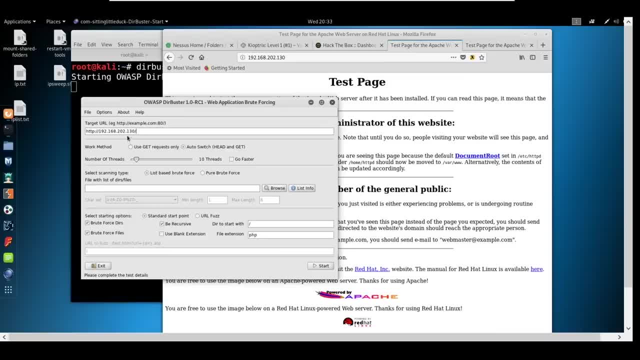 It doesn't really matter, Just paste it into here. Make sure you have the correct syntax HTTP, and then I'm going to put the port 80 like it has. It asks about number of threads. I always click, go faster. And now it's asking us for a file list. So it wants to be able to know what sort of 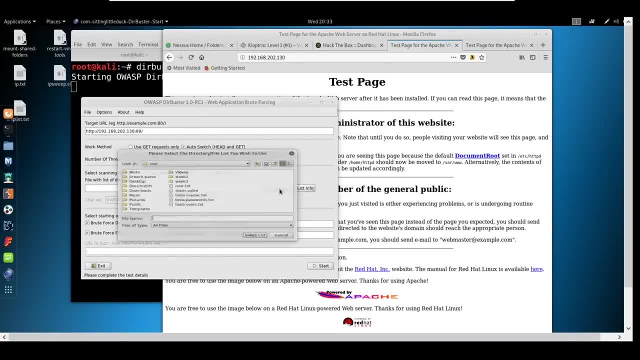 word list. it's going to run through And I'll show you where the common word list is. So if you click on browse and you say, look in, we're going to go back a directory And we're going to go to user, We're going to go to share, right here. 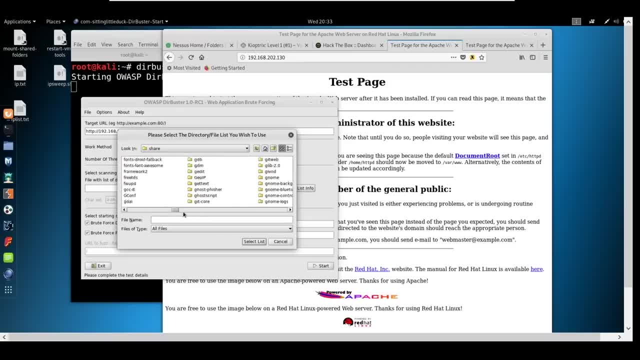 We're going to scroll all the way over until we see word list And there is a folder in here called Durabuster. We'll just double click on that And we've got options in here. So we've got quite a few. 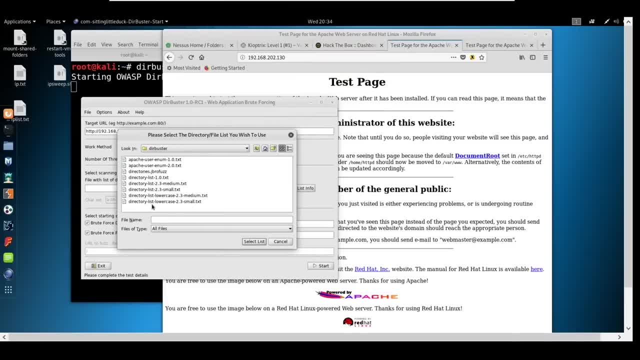 Just for proof of concept, we've got this directory list. lowercase small. This is plenty. We could run the medium. And if we actually went out to GitHub, there is a large version as well. I've used the large version on assessments, where I've got quite a bit of time just to run that. 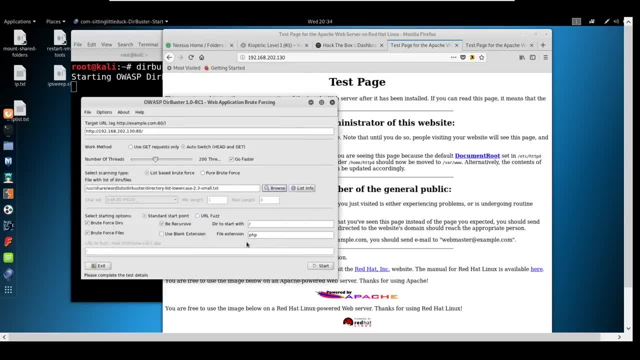 So we'll just go ahead and select this small here. Okay, So we're going to brute force directories. We're going to brute force files. We're going to be recursive. Make sure, we're going to do that. So we're going to do that. We're going to do that. 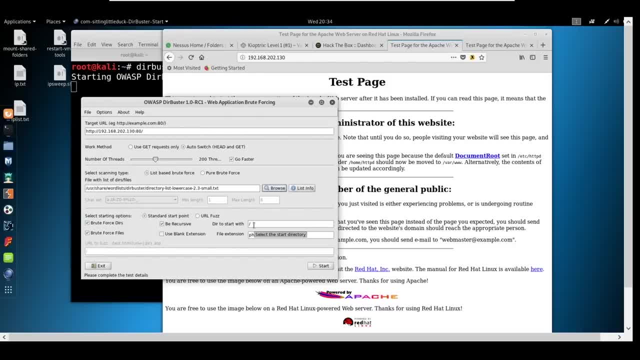 We're going to be recursive, meaning if we find a directory, we're going to try to scan that next directory as well. And now it's going to ask about file extensions. So we know we're running an Apache server, So we're going to be using PHP as a file extension. If this were an IIS server. 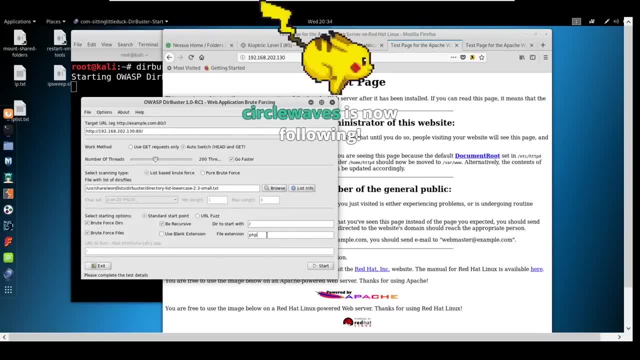 we'd be using ASP, ASPX, ASM, ASMX, those types of extensions. On top of this, outside of this PHP, we should look at other things as well. So we should be looking for any kind of interesting file that would be there, So we could say PHP, We could say ASA, What else? SQL zip file. 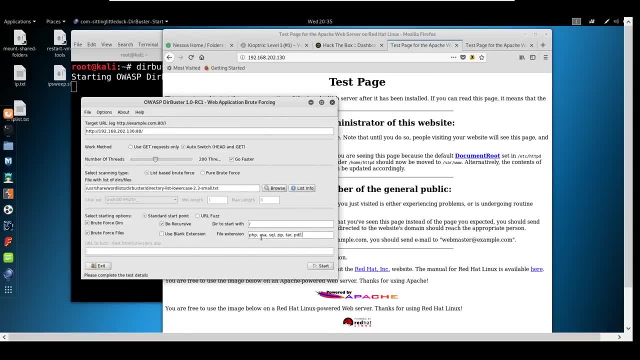 ATAR file. PDF text file, back file. This adds right. So imagine, every time that we add something here, we are adding that list all over again. So we're going to go through the list for blanks, We're going to go. 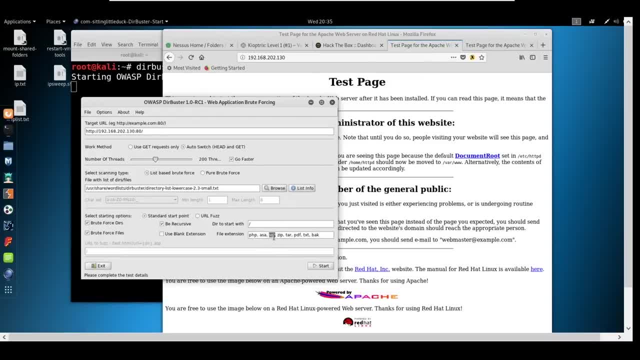 through the list for every single one of these file extensions as well, But it's always good to look through this just to see if you find anything of interest that's hidden out there. So we're going to go ahead and hit save. Start on this guy. 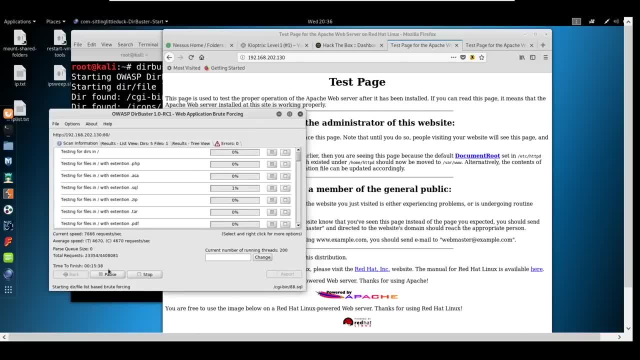 And that's going to run in the background. That will take some time. It gives you a pretty good time estimate here, So it's got 18 minutes And the more directories that it finds. you could see like it's already finding a list view If we click onto the list view. 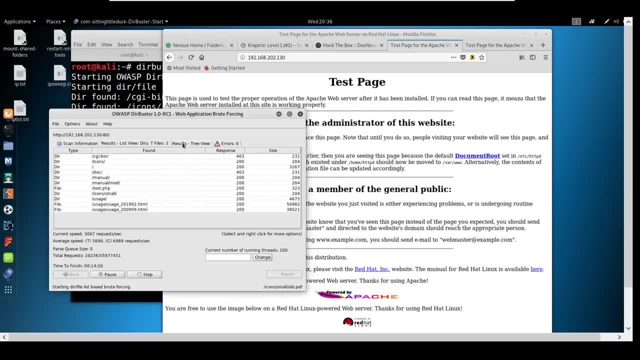 it's already starting to find directories And then if we went into the tree view, you can kind of look at it a little easier. So it's found this usage, It's found manual doc And it just depends what actually comes in here. So we could actually stop some of these Like: 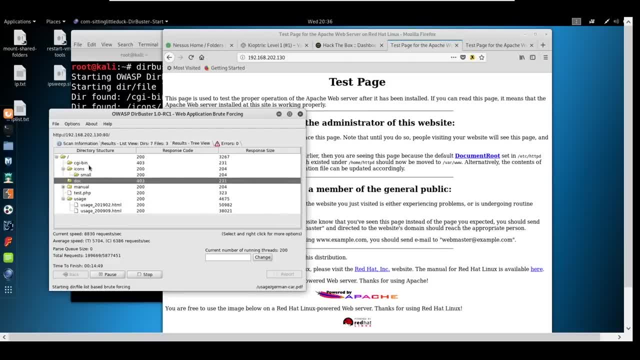 if we found icons, we could just stop icons or stop docs if we weren't interested in seeing that There's this usage page here which gave us a 200 response code, meaning that it's- you know, it's- a success. So we could open that in the browser and see what's there. 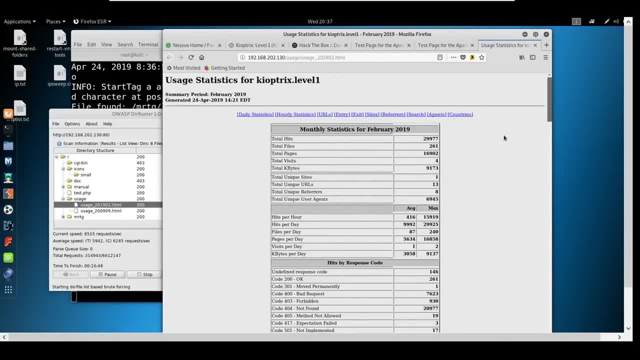 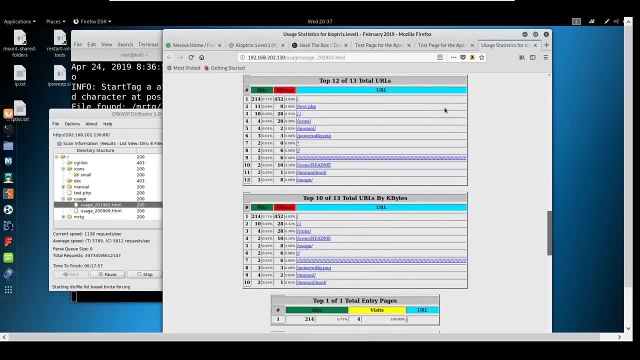 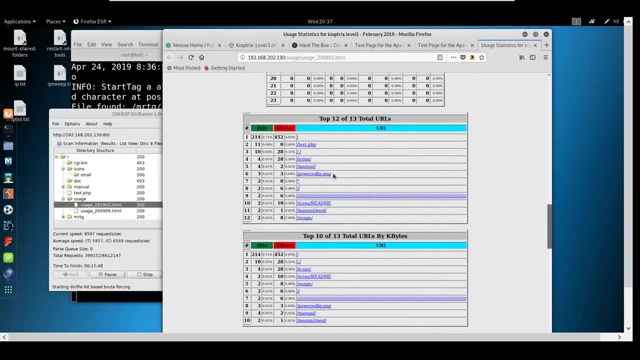 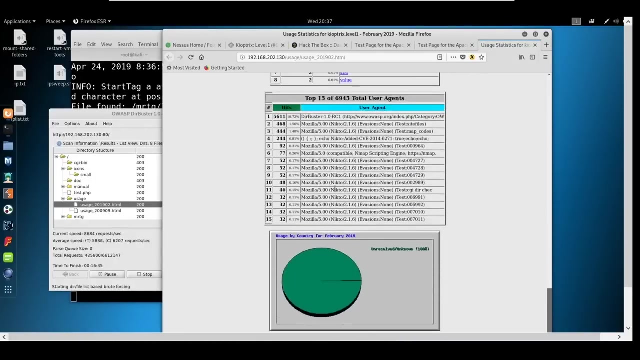 So it looks like they have some sort of monthly statistics on their page- Who knows if we're going to find this information or not- And then it shows you the different URLs that have been accessed here. So this is a little bit of information disclosure as well. So it would. 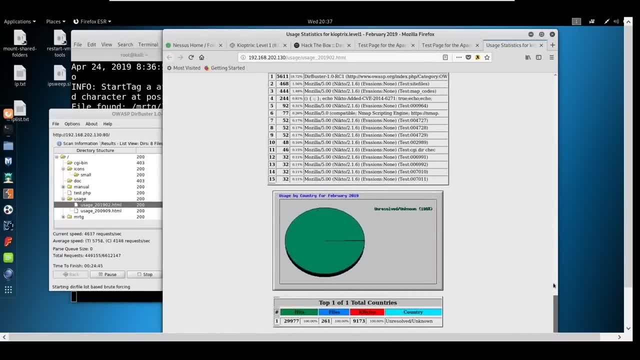 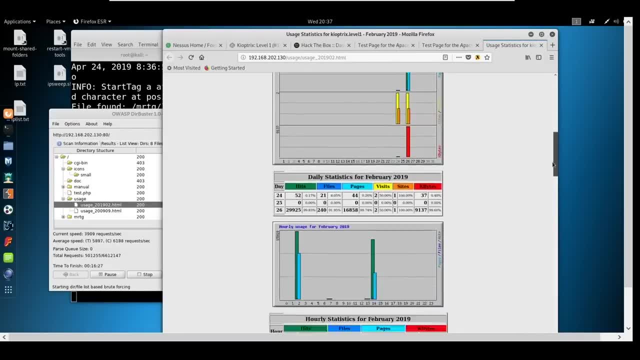 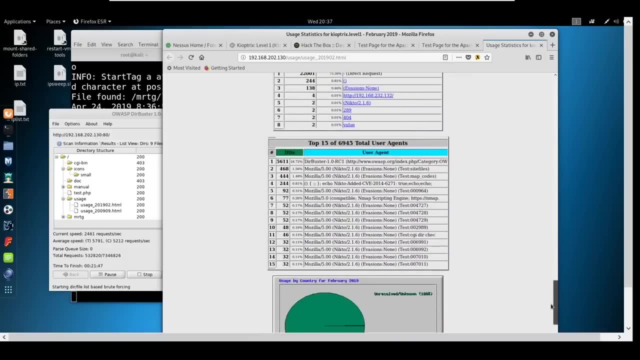 depend on what we actually found in this page, whether or not we would actually report this and whether or not this should be something that a non-administrative user should be able to see. My guess would be no, that you should not be able to see these sorts of things, But you would want. 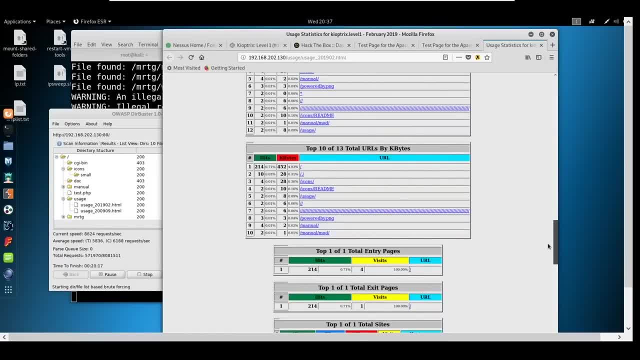 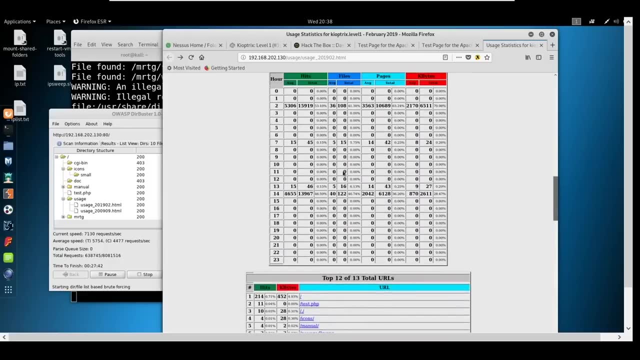 to talk to the. you know you'd want to talk to somebody on the other team and say: is there a reason? this is out on the web unauthenticated And they may have some decent reason for it. So you can see that there's pages here that came out with nothing, But so that's interesting. 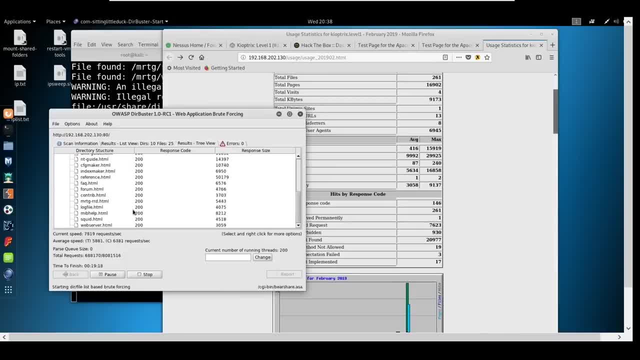 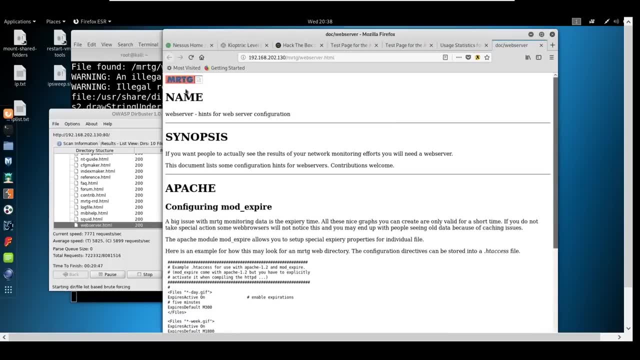 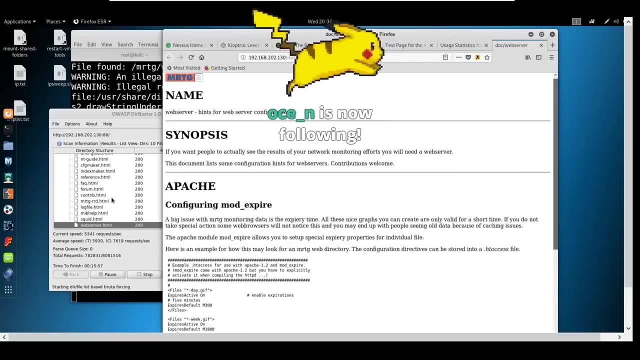 There's all these pages back here as well. There's a web server 200.. You can open that in the browser MRTG And we just keep digging and keep digging here, right? So we'll let this run and see what else comes up. 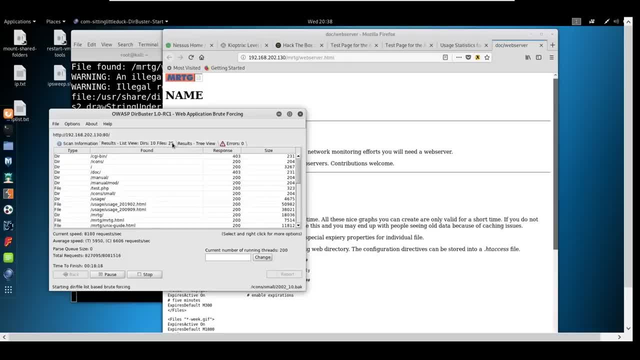 But the whole point in everything that we're doing right now is we're just, we're just enumerating, Right? So we're just, we're just, we're just enumerating. All we're looking to do is is dig as deep as we can until we can find any sort of useful. 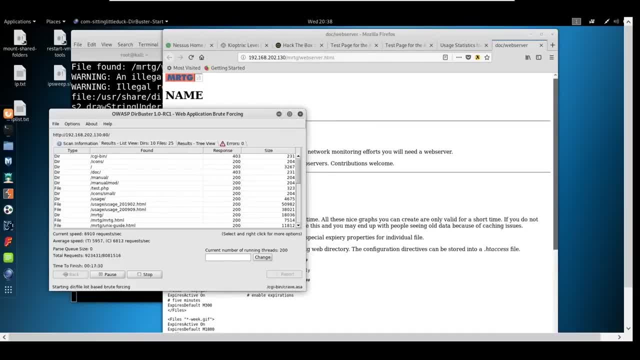 information And we're going to try to report on everything that we can find that is relevant. That way, we can improve the client security posture And we can feel like we did a good job as well. And thank you for the sub. I just saw that come through. I appreciate that. 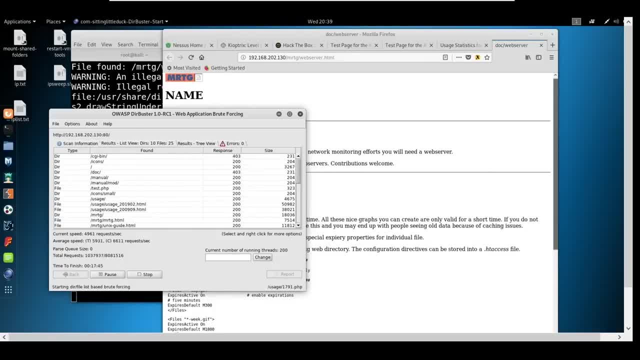 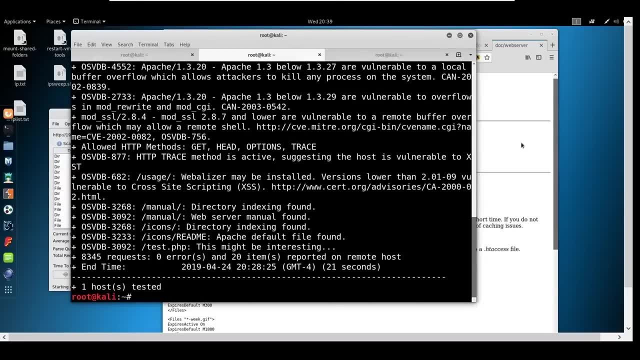 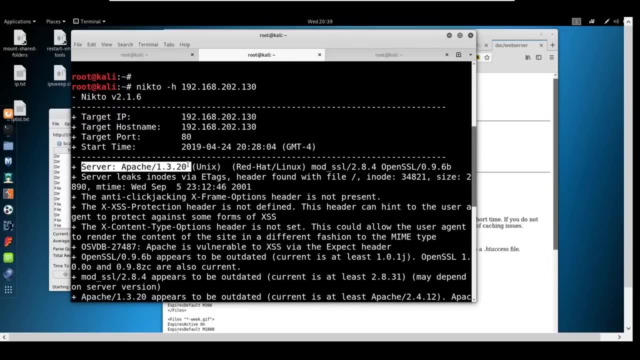 Okay, So while this runs, let's go ahead and take a look at something. So we've seen the server header pop up a few times. I actually kind of want to look at that. I just want to see what the response. 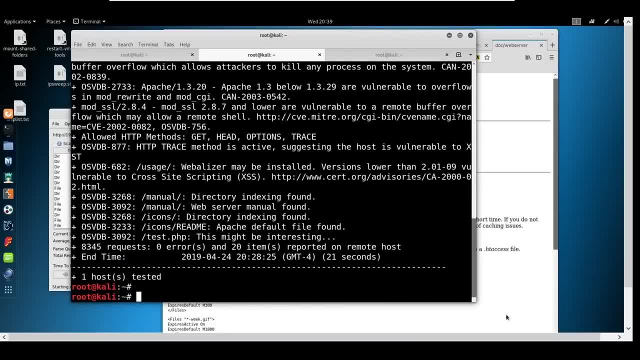 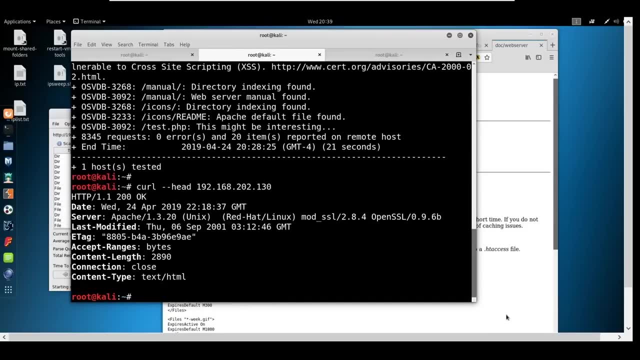 header is when we make a request. So let's go ahead and just use. we can use a tool called curl, We could do a dash dash head like this And we could say 192.168.202.130.. Okay, So now we've got some some disclosure here. Information disclosure- right. 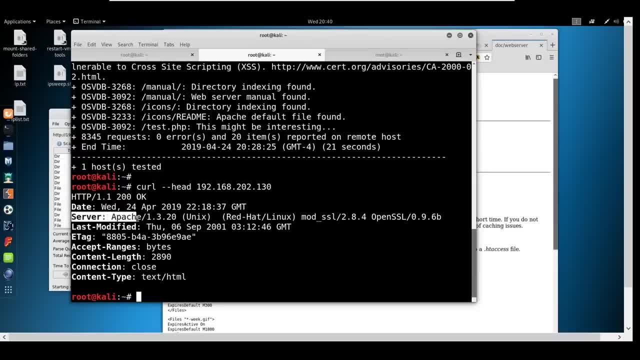 We absolutely have a server tag in here. server header in here with Apache listed. We've got the mod SSL as well. We've got the server header in here with Apache listed. We've got the mod SSL as well. We've got the server header in here with Apache listed. We've got the mod SSL as well. 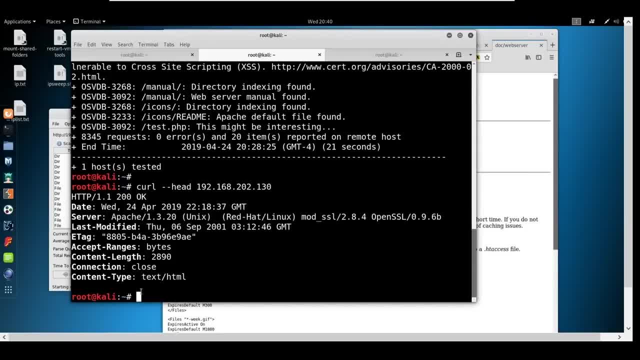 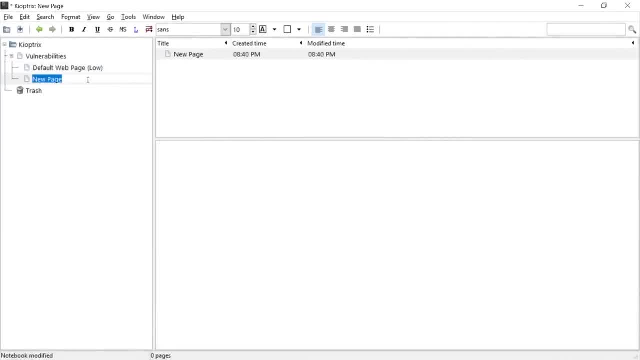 You know, this just keeps coming up. So what we're going to do is we're going to take a screenshot of this and we're going to report this as well. So let's go ahead and just do a new page and we'll say: server header info- disclosure. 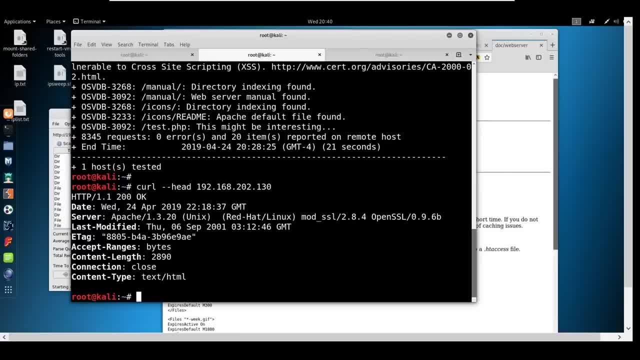 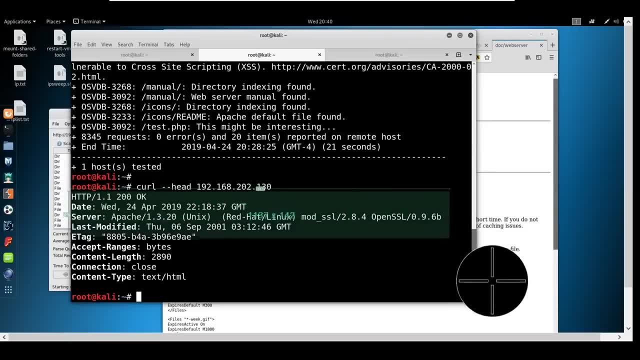 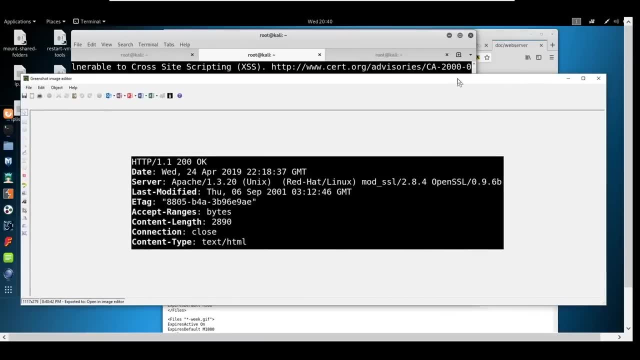 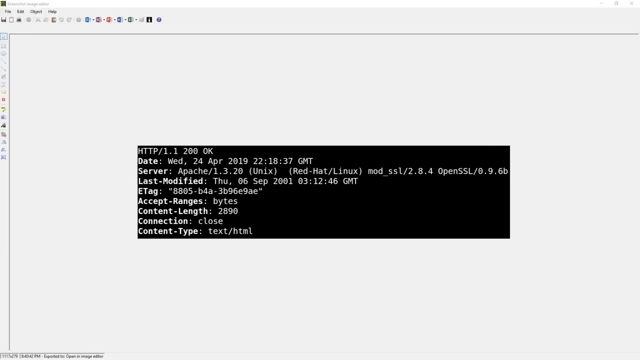 Copy that, paste it, And I'm going to show you a new trick with this. So, once we get this screenshot, let's open this in image editor. I'm going to bring this over, All right, For the purpose of making our reports look good and for the purpose of not wasting ink. 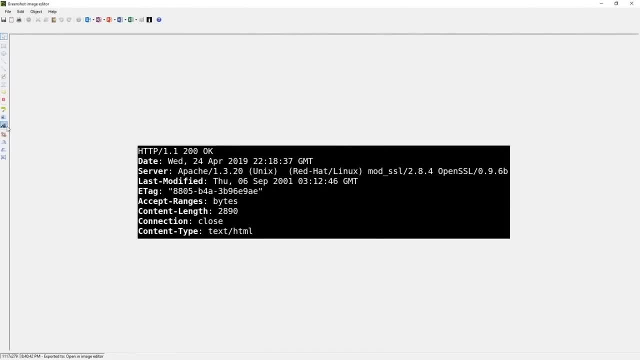 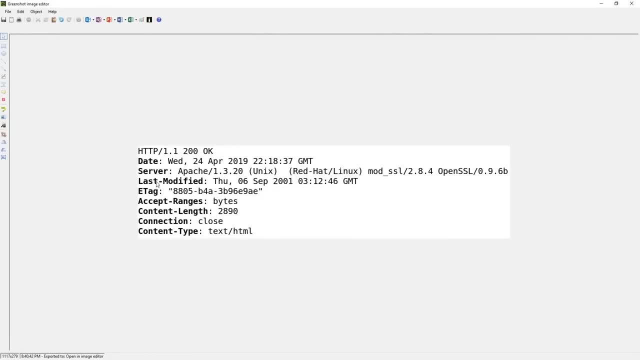 this black background here is awful. We can come into this little tab over here and say invert, And then we can turn that into white. This looks much, much better on reports. It saves you ink. It's an all-around win-win. 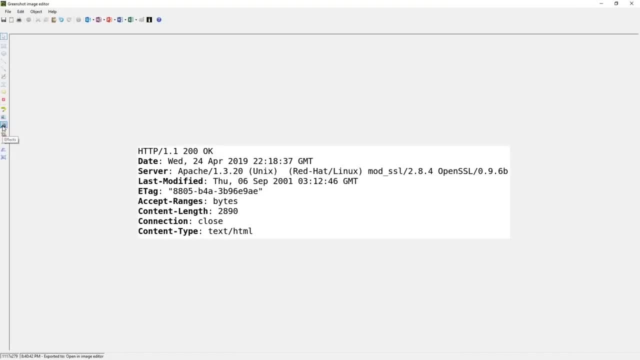 So nifty little trick right here on the little magic hat: Faxes as well. Somebody said: if you're faxing your reports, I would probably highlight this server here. Also, E-tags. while not serious, This is an information disclosure that we can highlight. 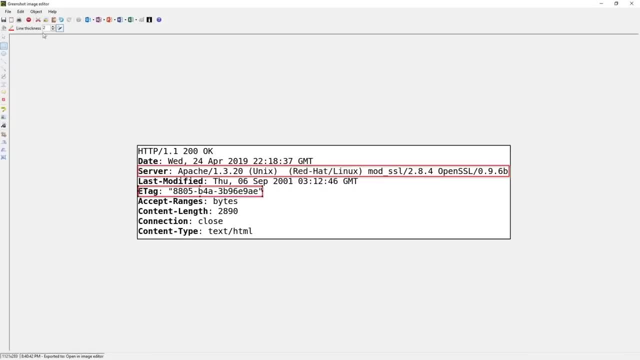 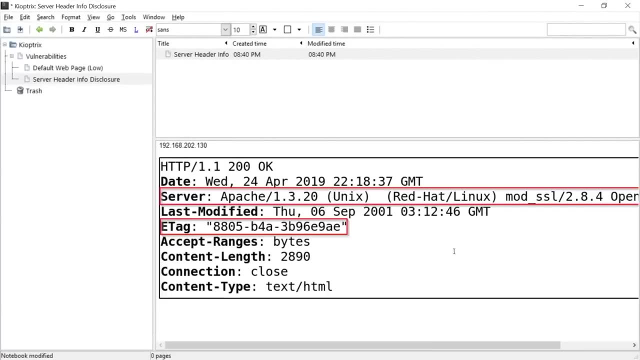 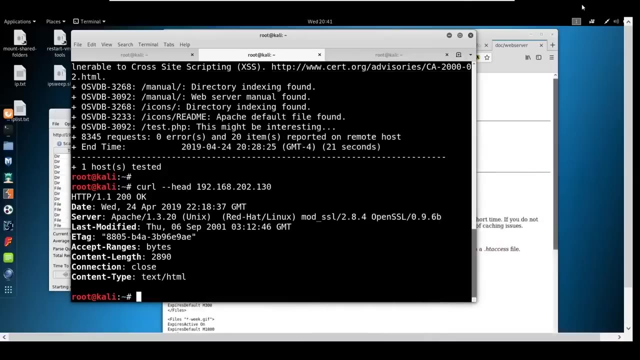 As always, I like to put my pretty little border on it And we'll say: copy, come into here and we'll paste this information. Okay, So I saw a comment come through saying that we should check for error pages as well. 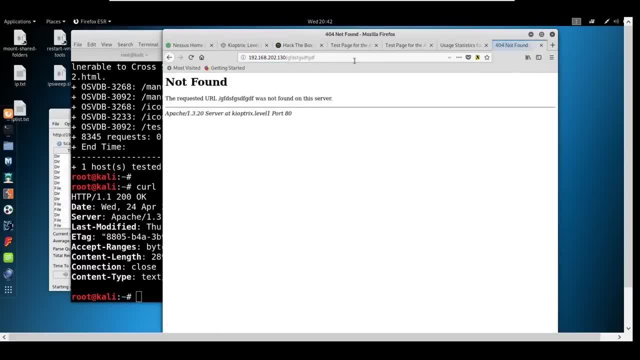 I agree. So you come in here 404, and what do you know? There's another finding. So on top of the header disclosure, they're also doing information disclosure as well with their 404 page. They're using the generic Apache 404, not found, instead of having their own 404 page. 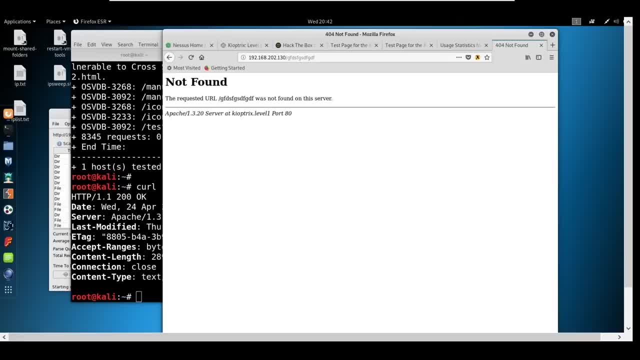 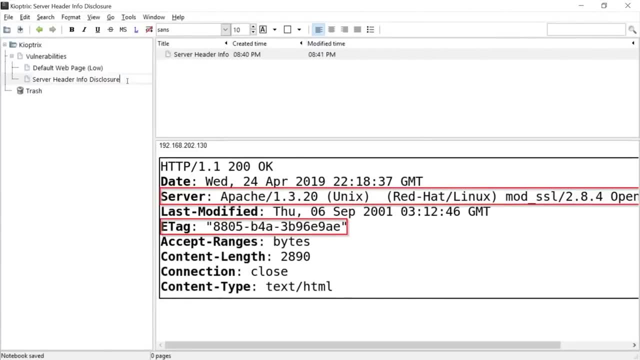 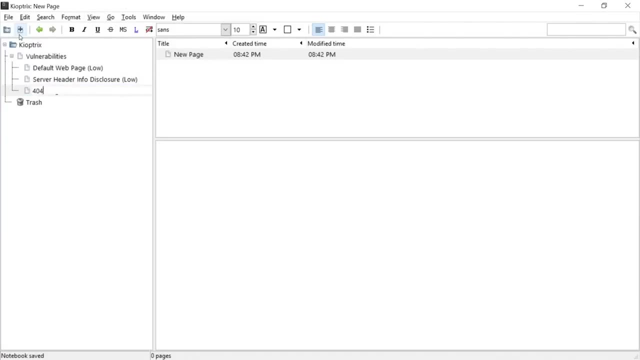 So this as well would be a finding. So we'll come back into here. make another finding Also: this info disclosure is all. this is low. We'll say 404, default 404, info disclosure And, honestly, when we come through here, 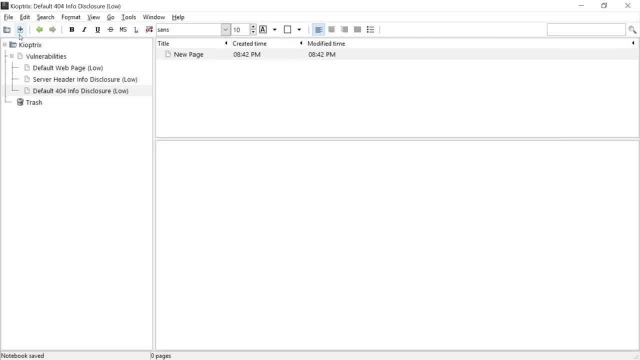 Okay, When we come through here and we have enough info disclosures like this, you might just throw them into one finding altogether. So it depends if I've seen it where, if I've had a bunch of them, I'll just put them into it. 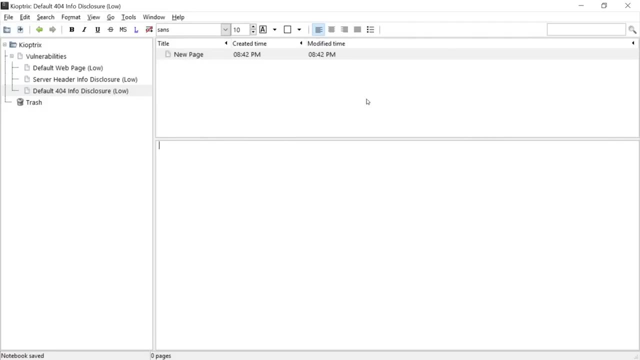 If I've only got like one or two, I'll probably make them separate findings. But if they're doing it all over the place with information disclosure, you might just throw it in and have a bunch of screenshots of all the locations they're doing it. 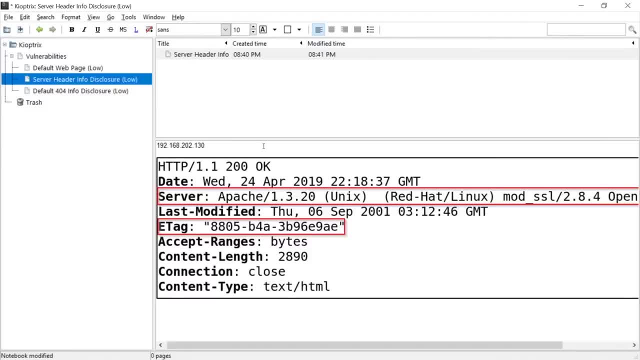 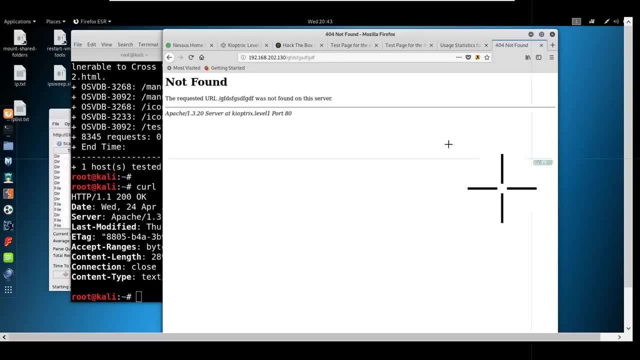 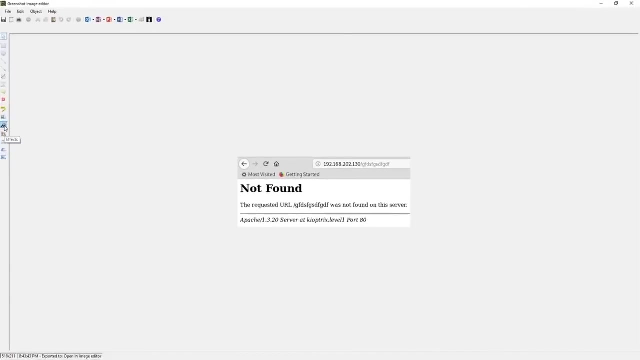 So it just depends, Okay. So again, we'll copy the IP address, just to be consistent, And we'll take a quick screenshot of that. Bring this over again And we're just going to put a border and just copy this. We could highlight down here the disclosure as well. 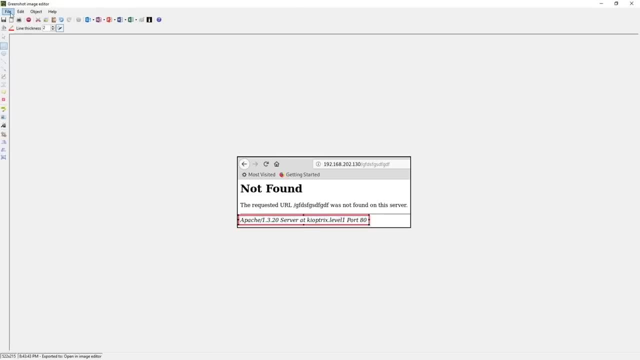 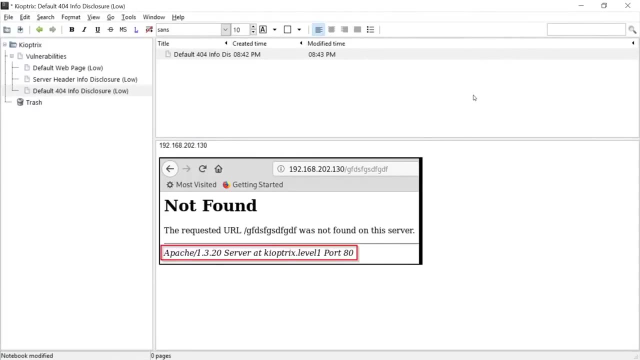 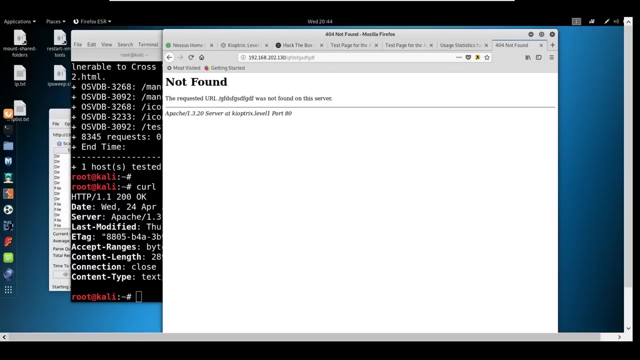 Okay, So we'll just drag and drop, Copy and paste. All right, So now, what else can we look into Before we dig into the heavy hitting stuff? Okay, I want to show you one more thing that we already covered last week. 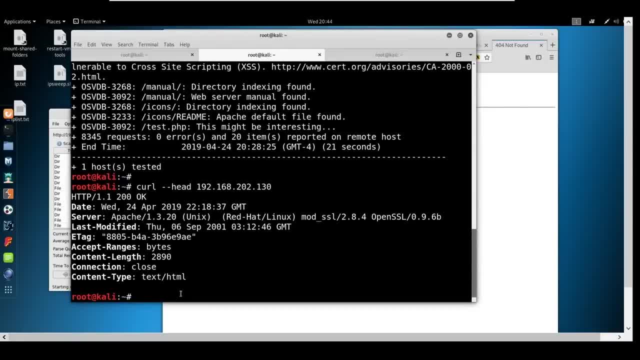 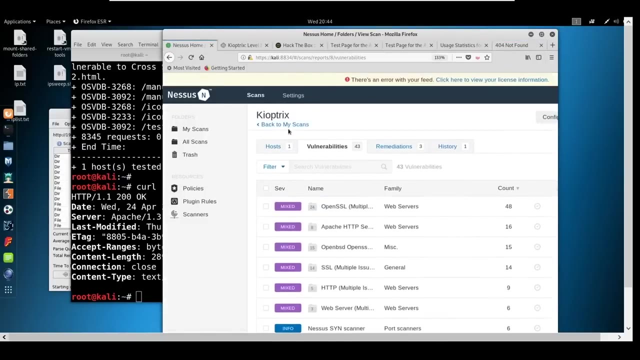 And then we'll start digging into the heavier exploity type things. All right, So last week we talked about Nmap and we talked about ciphers and certificates. When we come into Nessus and we looked at this, Let's see if this scan is done. 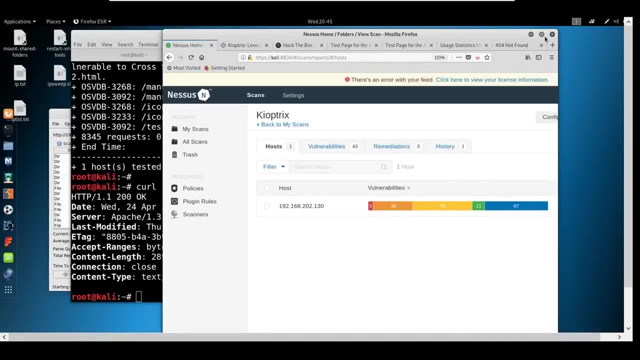 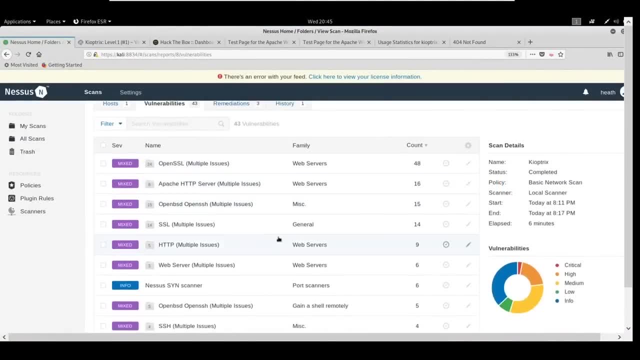 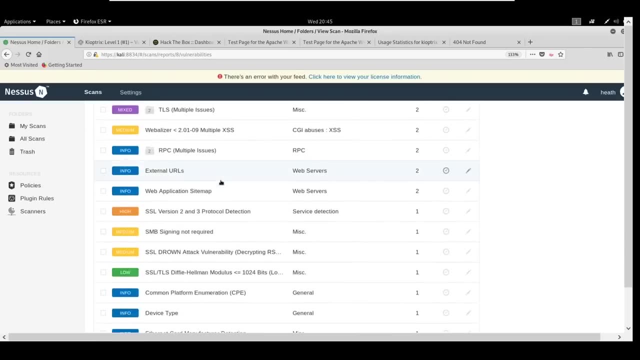 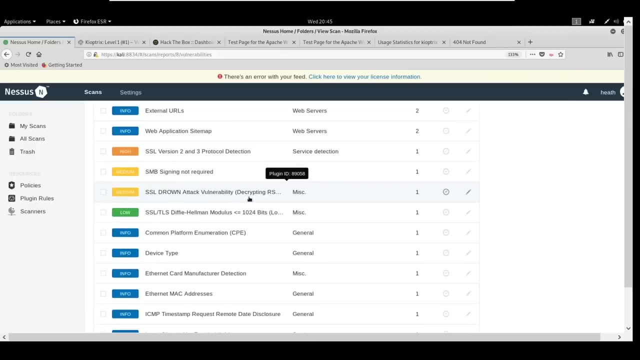 Yeah, we are 100% on this. Okay, So we come into here and we'll see that there's a lot of issues with certificates And you can kind of come through like: see this SSL drown attack. That's a sign or not certificate. sorry of ciphering. 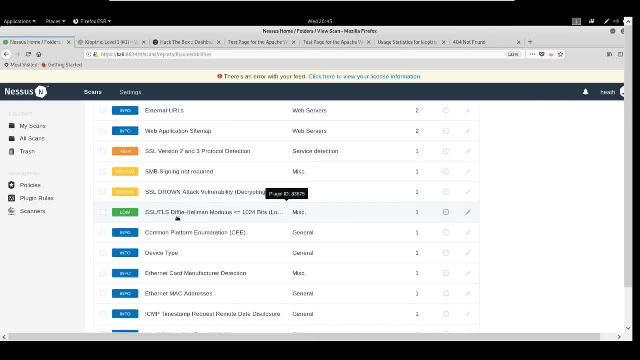 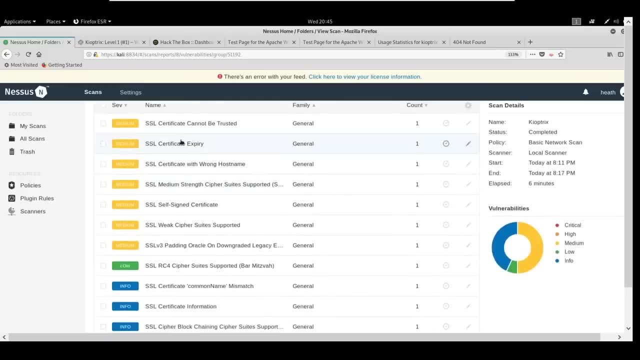 That's a sign of a cipher issue. This SSL, Even though it's a low, It's a sign of a cipher issue. If we click into some of these like this SSL here certificate cannot be trusted. expiry- wrong host name. 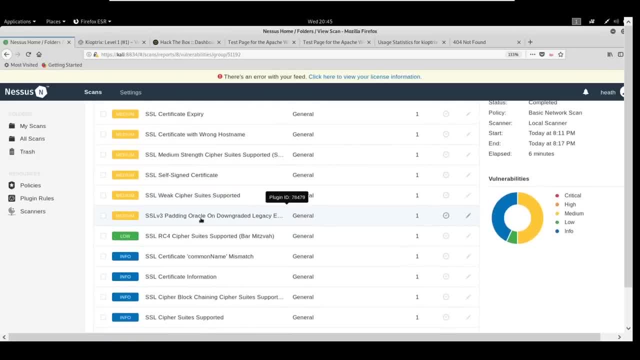 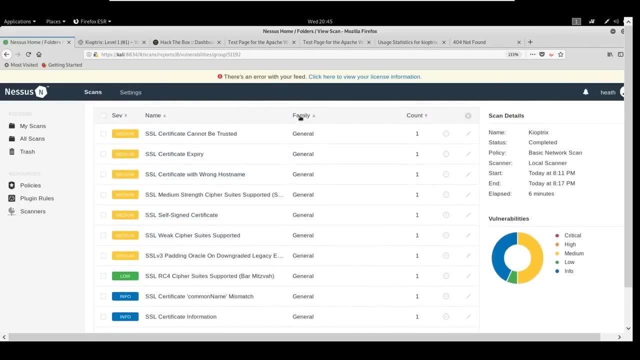 There's all kinds of certificate issues that we would look into. You would look into some of these other ones as well, like the weak cipher suite supported the bar mitzvah Poodle's, another big one, etc. So we're not going to go too heavy into those because this is just overwhelming with them. 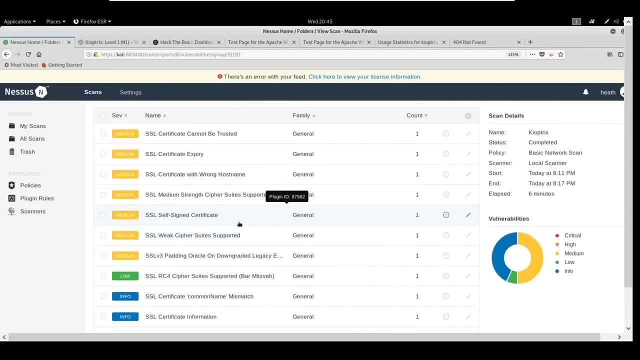 But I'll tell you what we do in terms of finding. This is absolutely a finding and we're going to just kind of use a generic way of reporting this tonight. But what we've built out is an Excel document, basically, that we can parse Ness's into, and 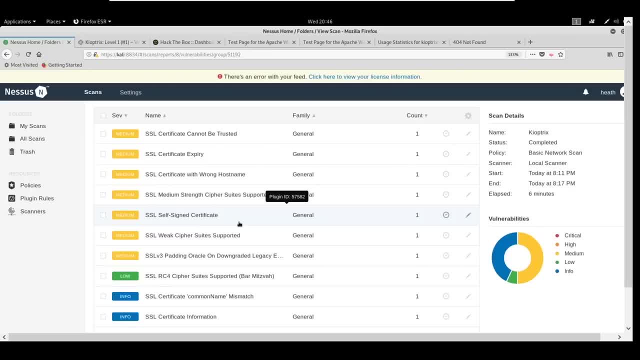 then it reports back all the SSL issues for all the servers that are out there, the web servers that are out there, and gives you a nice overview, because a lot of these attacks like Poodle or bar mitzvah, It requires some sort of man in the middle. 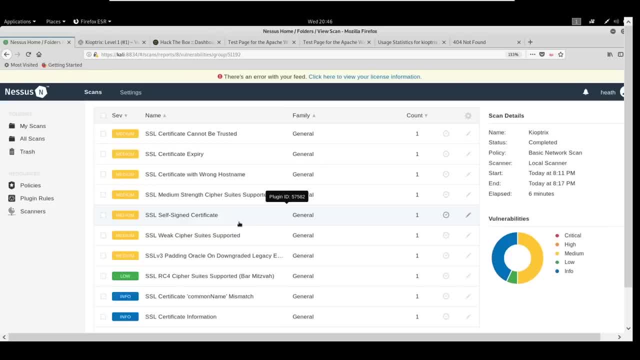 They require an extensive amount of time and they're just not easy attacks to pull off, So they're not something that you would typically go after in an assessment, but they're definitely things that you would notate in an assessment because you're not going to waste. 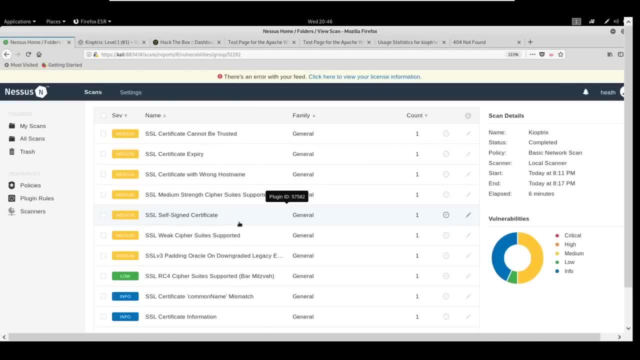 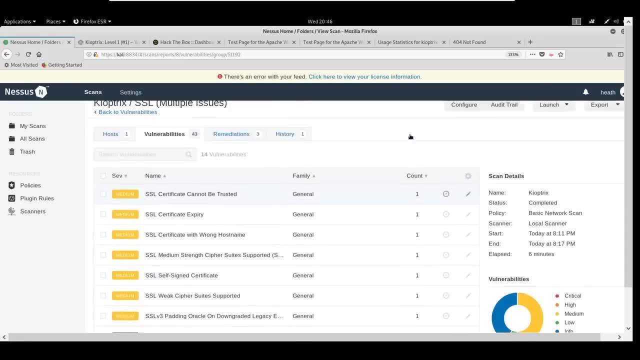 If you're given 40 hours, you're not going to waste all your time trying to do a man in the middle attack on an external assessment, if that makes sense. So the one way we're going to notate this, Okay, Okay. 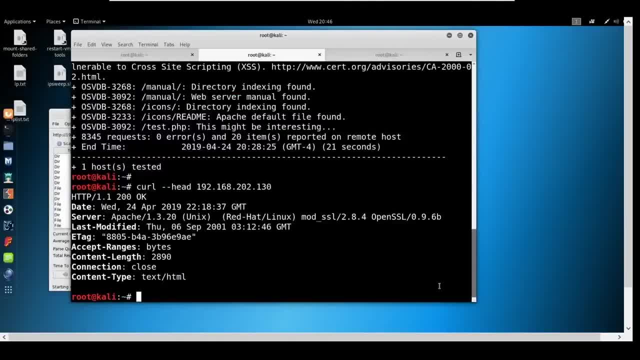 So the way we're going to notate this is: we're going to use Nmap, And there are websites out there that do this for you, like Qualys SSL does this for you If the site is live. but the site is not live. 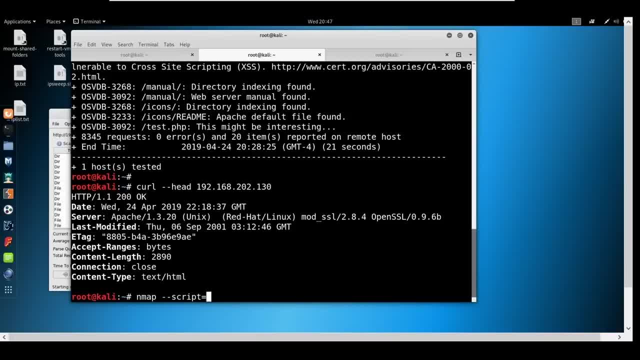 And I actually like the. I like the Nmap output better, but I've seen it go both ways All right. So the script that we ran last week was this guy: Nmap dash. dash script equals SSL enum ciphers, port 443.. 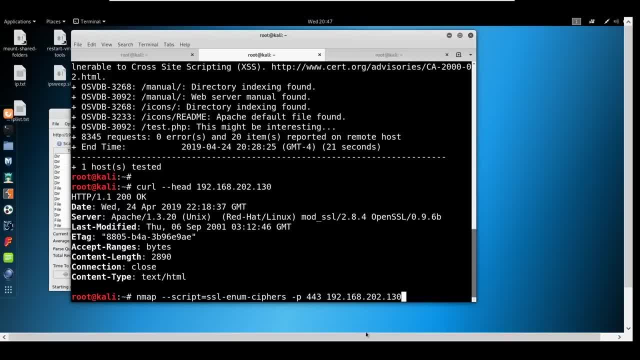 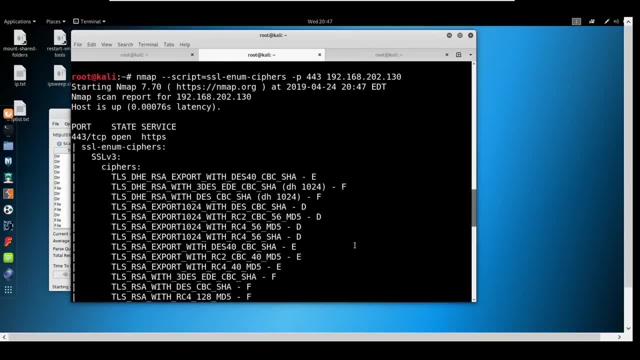 Then we're going to say 192.168.202.130,, hit enter. It's going to come back with all the ciphers. Now, Keoptrics is an old box. When Keoptrics came out maybe these ciphers were on the AI. 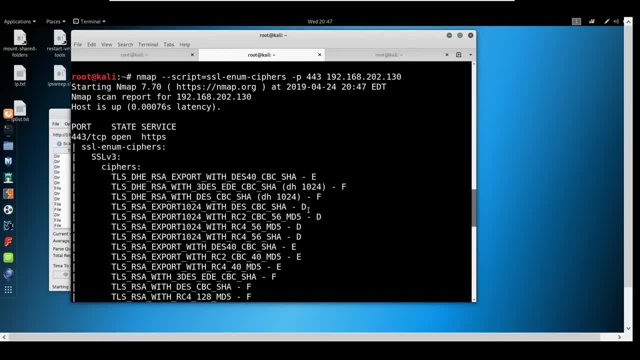 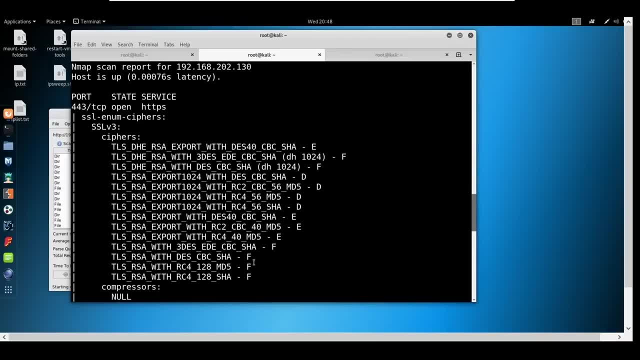 Side of things. But now, seeing that it's so old, these ciphers are deprecated, And last week when we looked at this, we looked at Tesla and you saw that Tesla was nothing but A's. You see here that it's mostly F's. 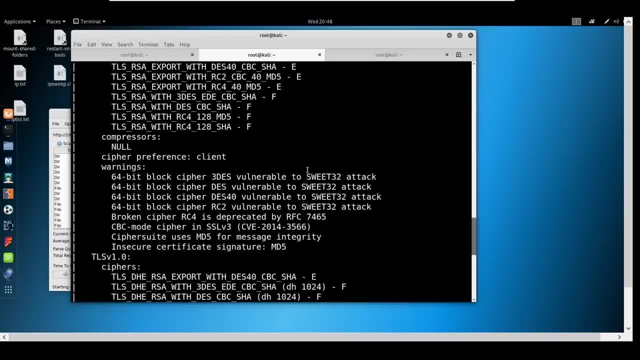 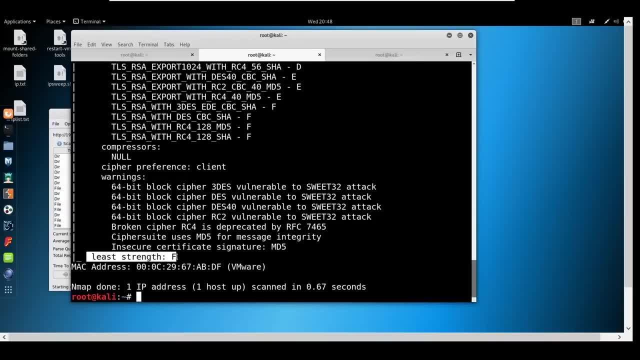 So the best one that they have looks like like it's a D, And if we scroll down to the bottom, what's really important to capture is the, the cipher, at least strength, And we'll- we'll basically just grab that. 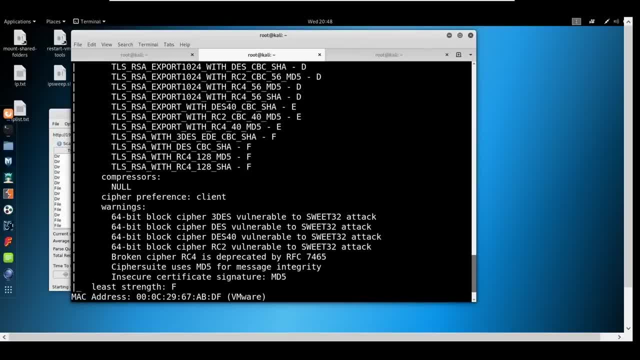 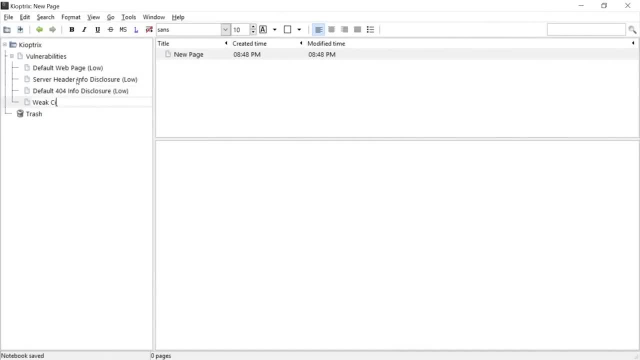 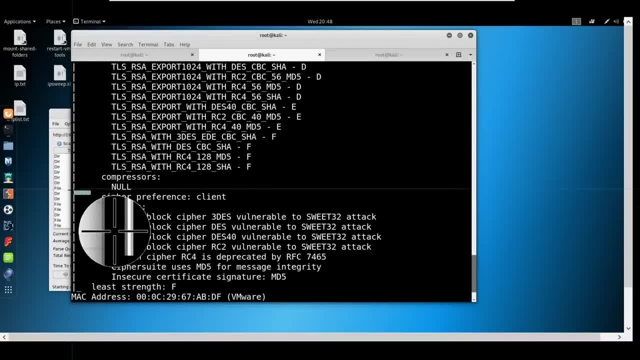 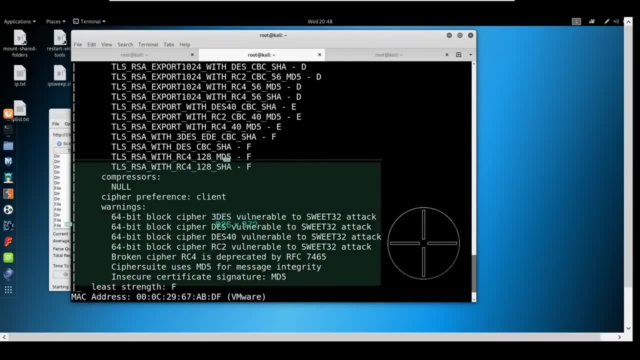 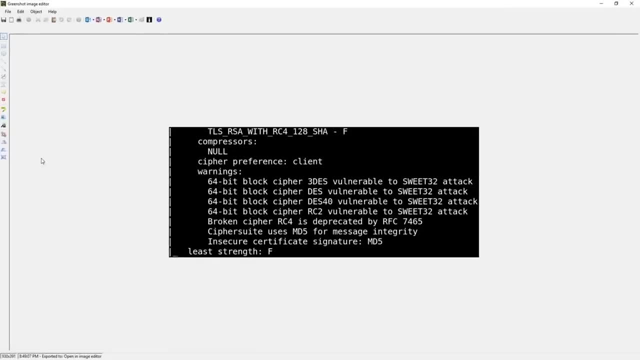 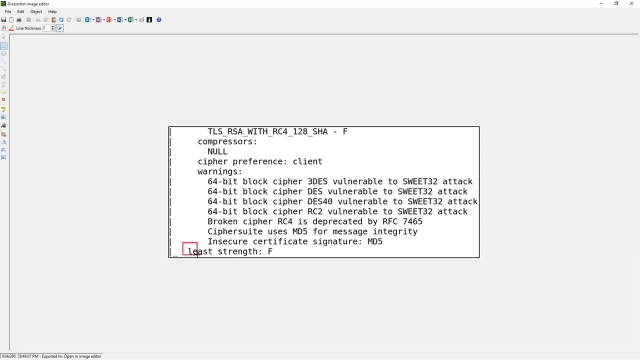 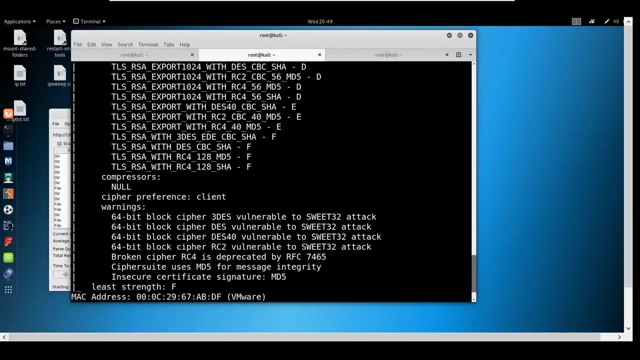 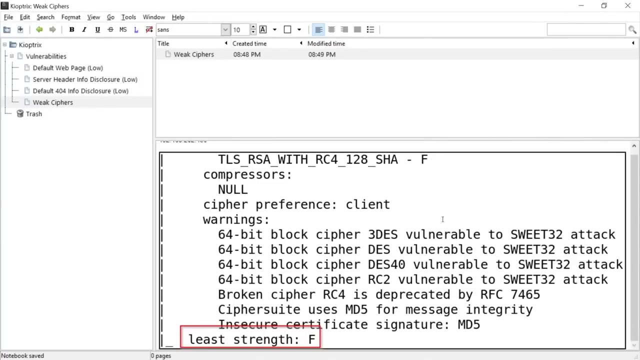 We'll just make a new one. We'll just make a really quick screenshot. Come in here. we will invert it, border it, capture the least strength as an F Copy. that Okay, And as I said before, we typically will report this a little differently. 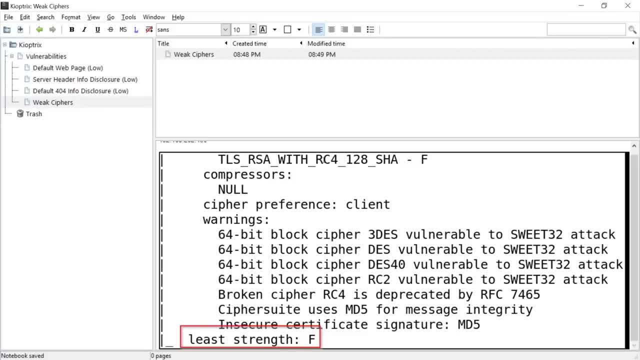 We'll do this on a web app assessment. if we're reporting a Qualys or this least strength via Nmap For an external assessment, especially if we've got a bunch of web servers that we're looking against, we'll build out a chart and it's a lot prettier. 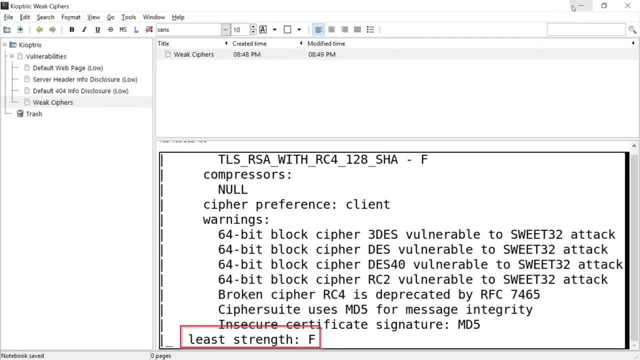 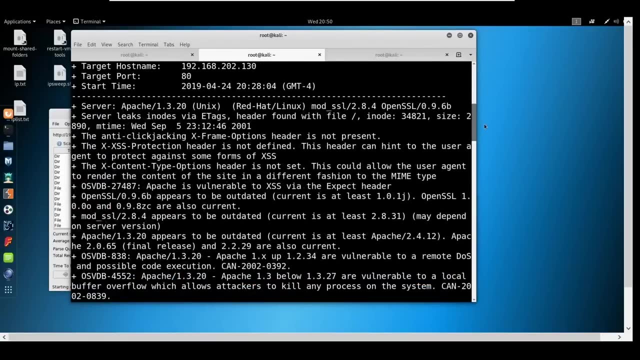 Unfortunately I can't show you that chart because that's a nondisclosure on my behalf, but just know that you can chart these all out, All right. So from here let's just go ahead and dive into the weeds. I'm going to take a drink, really quick. 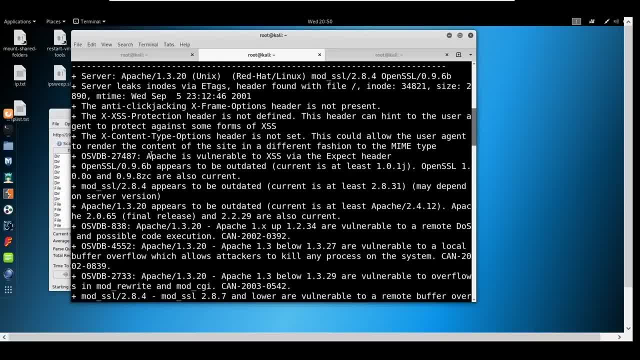 All right. So we've got a few things that we see. We've seen this Apache 1.3.20 come up a bunch of times. We've seen ModSSL 2.8.4 come up a bunch of times and this OpenSSL as well. 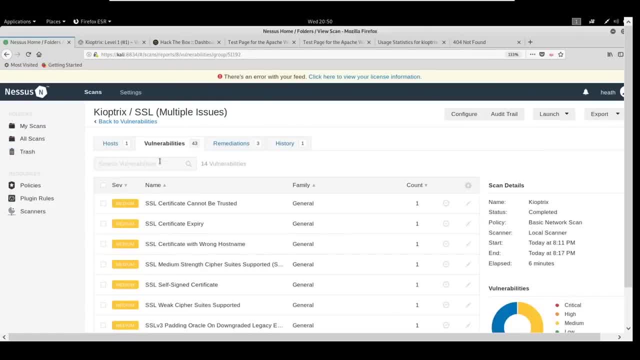 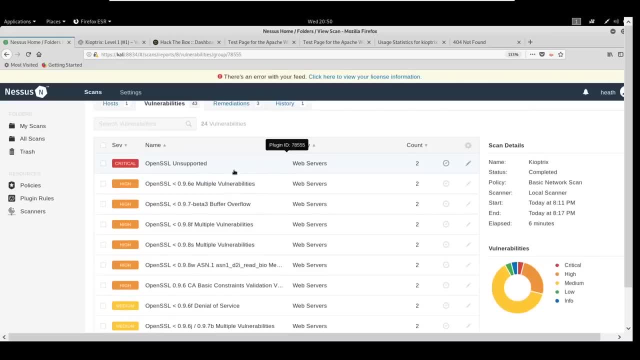 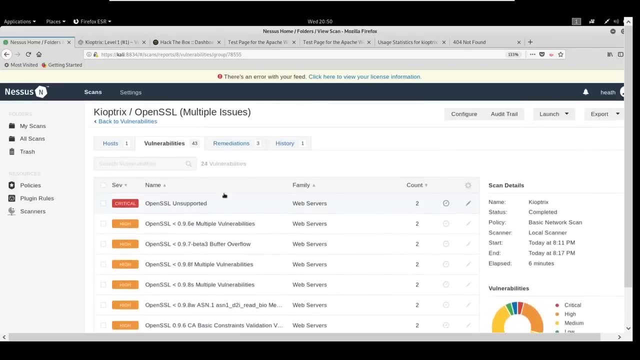 If we go into our Nessus scan, it's all over the place in there. OpenSSL has a critical vulnerability and it's got several high vulnerabilities and medium as well, So we can assume automatically that this OpenSSL version is outdated, has lots of vulnerabilities and is going to be something that we're going to be reporting on. 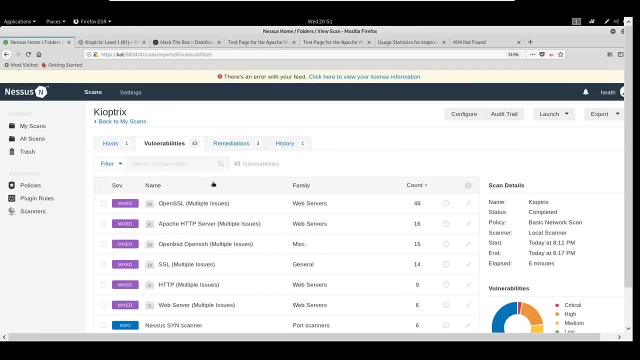 So, depending what we find is what we're going to report. As of right now, we haven't exploited anything, so we don't know how we're going to report this. It's potentially that it's outdated, but we're not able to exploit, and we'll notate that in the report. 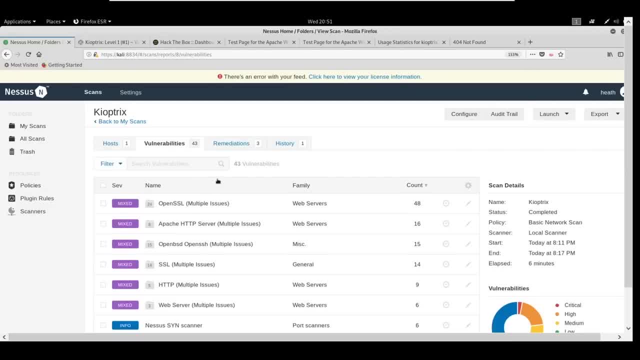 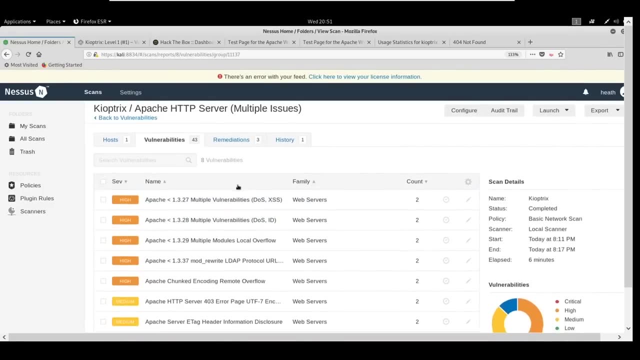 We'll say, hey, it's, It's outdated, You need to patch this. but we are unable to actually achieve any sort of exploit with this vulnerability or this outdated software. Same thing if we look at Apache. It looks like Apache has several issues as well. 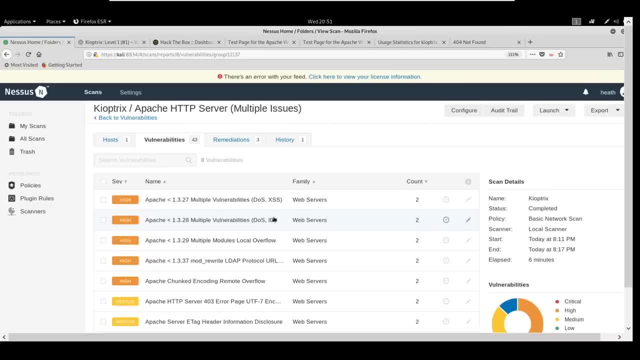 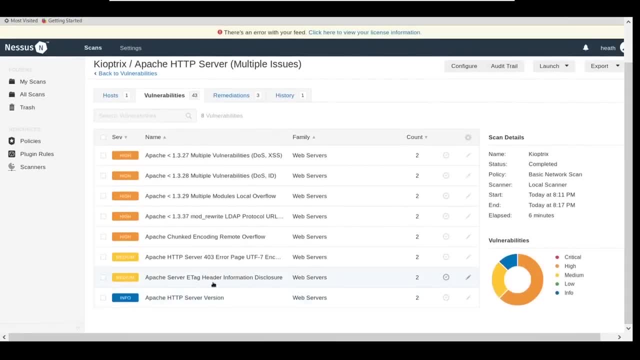 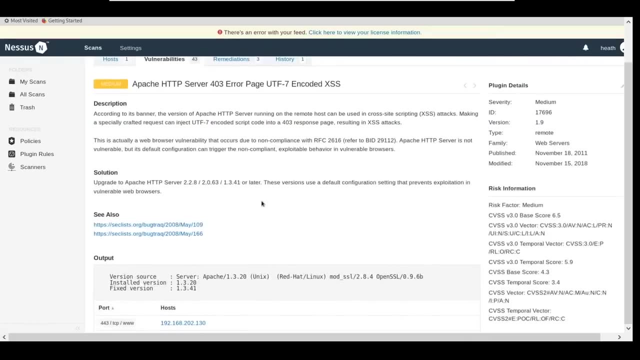 Just from the Nessus scan itself. it's got denial of service, cross-site scripting, a local overflow, a remote overflow. It caught the ETAG information disclosure that we talked about. It found a 403 error page. So just some things there. 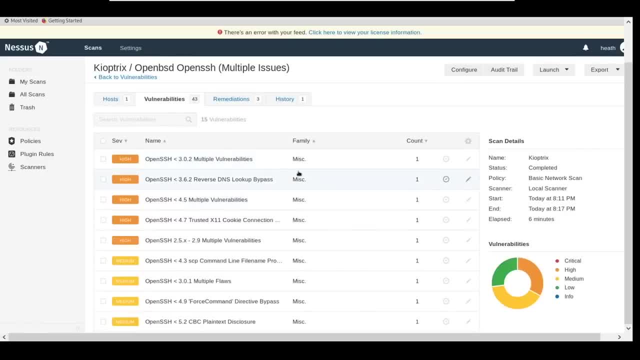 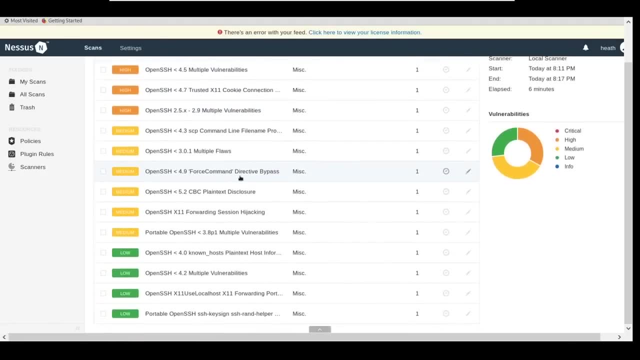 It's got some information on the OpenSSH, So it looks like this OpenSSH version they're running also has vulnerabilities. So that would be interesting. If we're doing an assessment of this company, our mouth is salivating because there's just so many things that are popping up. 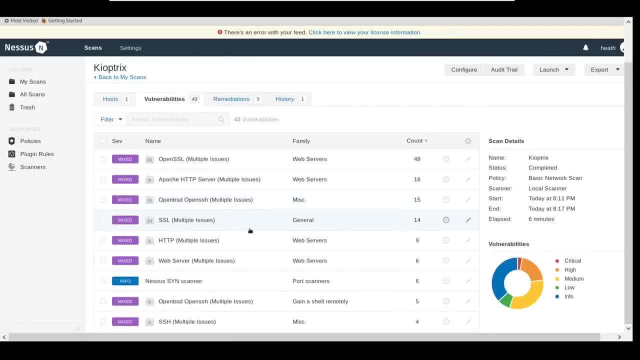 It doesn't mean that they're all valid. Sometimes false positives do show up, But when you see this many things going on through these reports, it really starts to get juicy. So look through there. There's some SSL or web server issues. 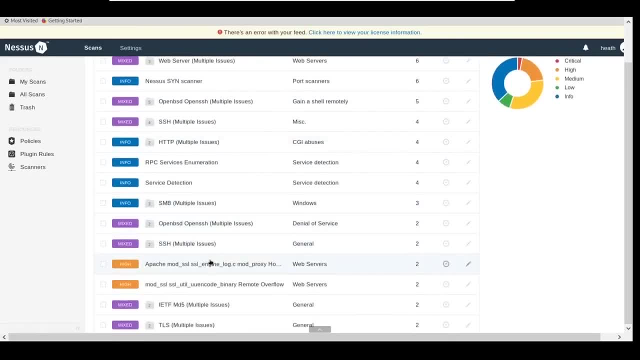 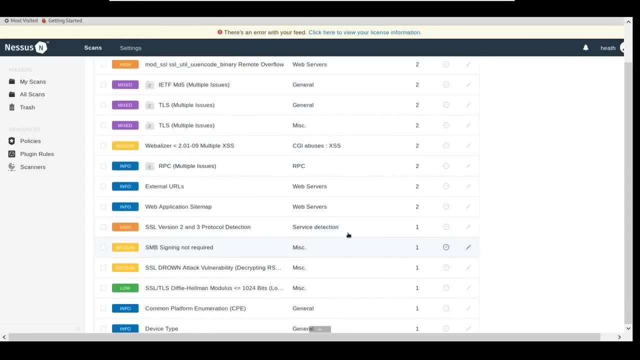 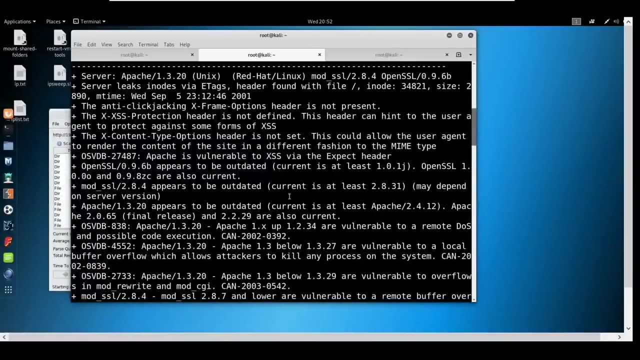 Again, OpenSSH, SSH, SSH, Apache Mod, SSL. So we'll dig through these as well if we're looking. But what I like to do, even with this sort of information, is I like to. I like to do it kind of actually on the manual side of things. 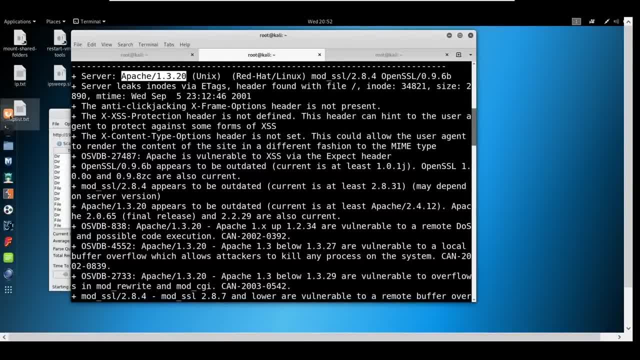 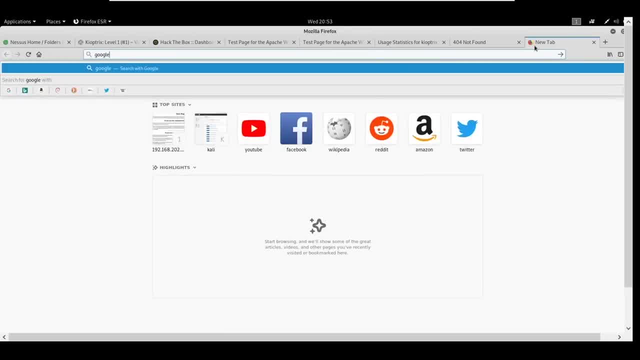 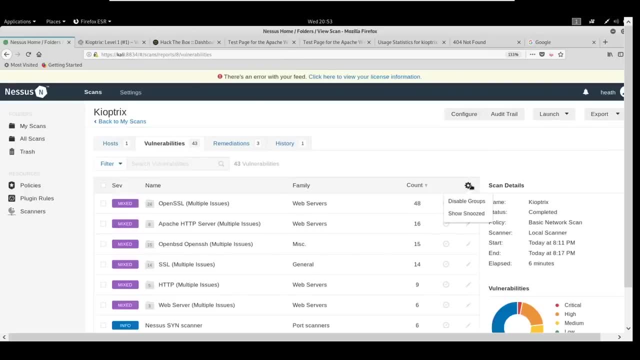 So if we've got Apache 1.3.20, for example, The first thing I'll do is I'll go out to Google. Somebody said the gear is: Ah, this gear Disable groups. Hell yeah, That's better. 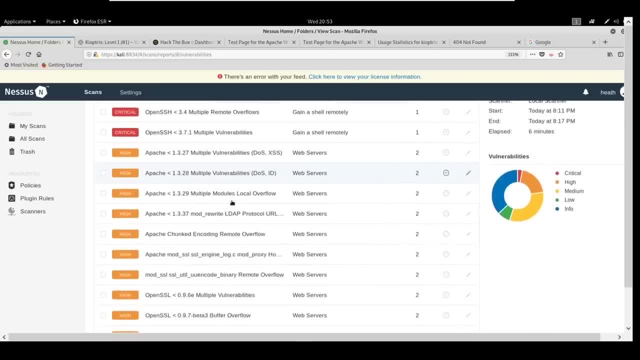 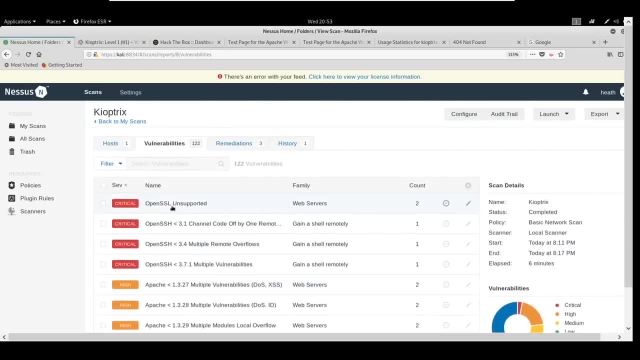 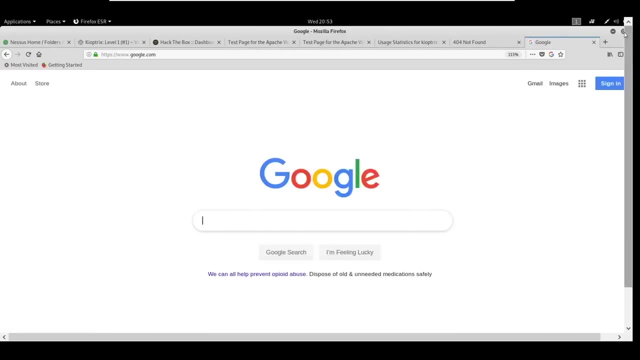 So we can sort by severity, And now you can see All All the issues that we really have with this server. There's quite a few, Mostly pertaining to OpenSSL or OpenSSH. Thanks for that, All right. So first one: we wanted to look at Apache 1.3.20. 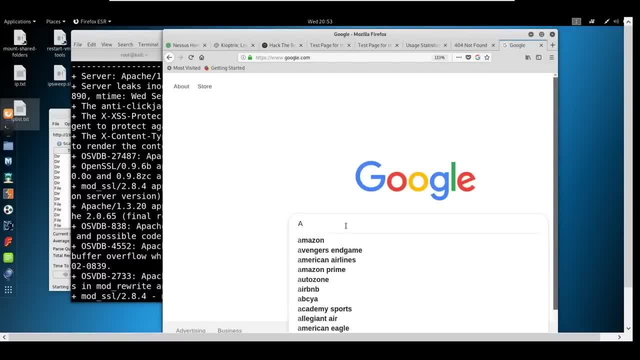 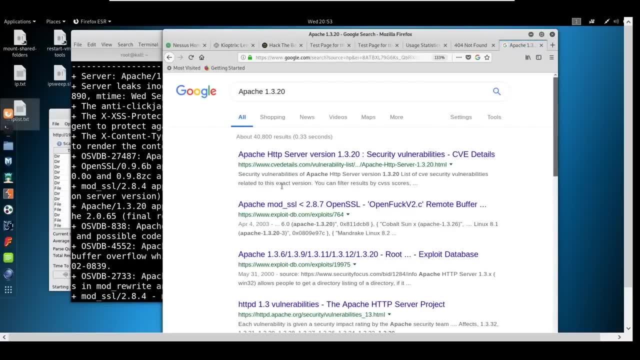 So, Okay, we're going to go to the API. We're going to go to the API And we can look up. We can look up the CVE details if we look into this. A great, great, great website that's going to become your friend if you stick into this. 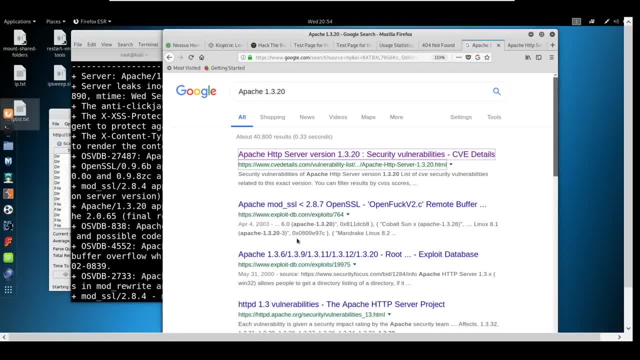 field is ExploitDB. It looks like somewhere in here it was mentioned, So we might open this as well, But this looks like it pertains to ModSSL 2.8.7 or less, And if we see over here, we do have ModSSL 2.8.7.. 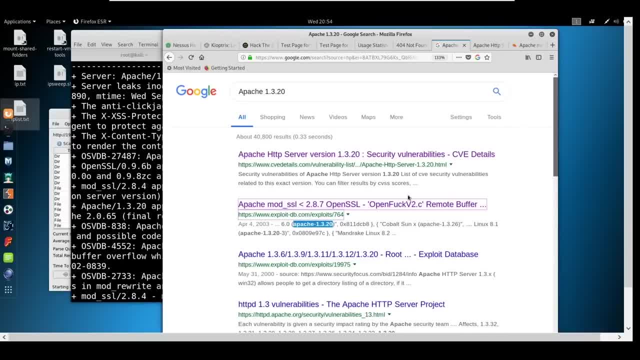 And this is the result of ModSSL 2.8.4.. So this may even be something that's lining up with multiple conditions. So if we see, okay, it requires Apache 1.3.20 and ModSSL 2.8.7 or less, then we're starting. 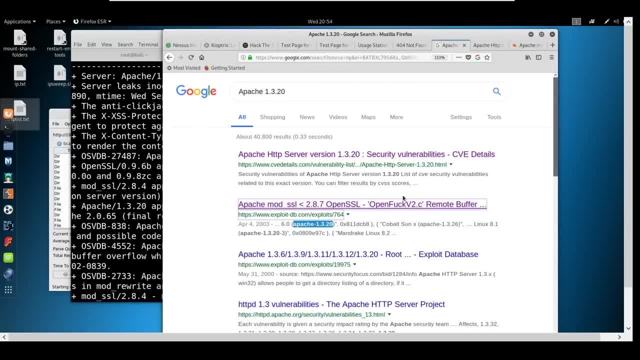 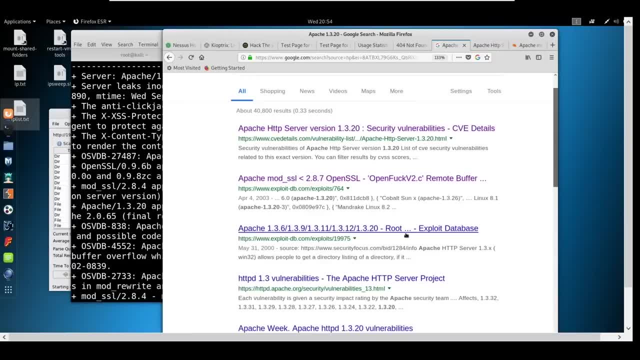 to meet those kinds of conditions Right. So this might be an exploit that we might be interested in Keep looking through here. 1.3.20. is another exploit, so let's start with the CVE details. I like to look by score. 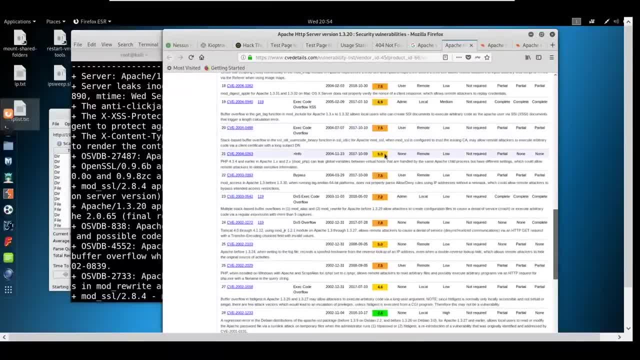 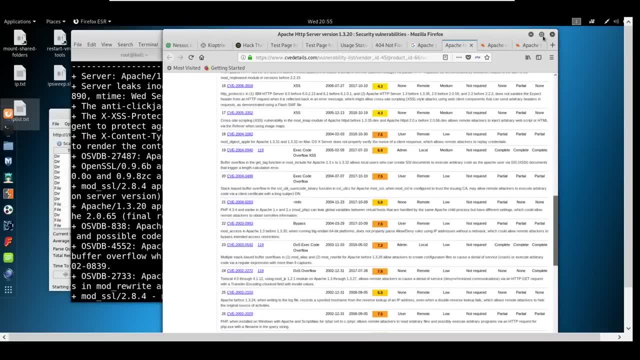 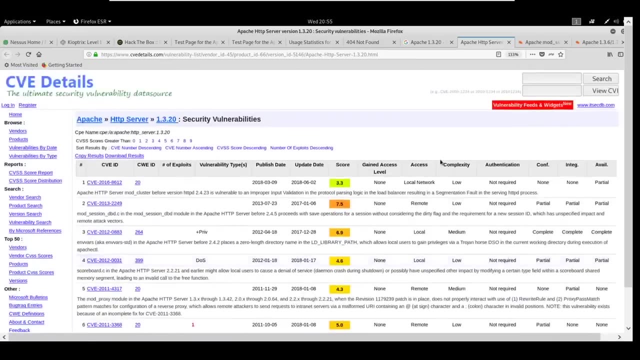 so the the higher the number, the better. it looks like there's a ton of vulnerabilities for this, so if we come into here, let me try to blow this up so you guys can see it okay. so we've got the score here and it's got the CVE by. 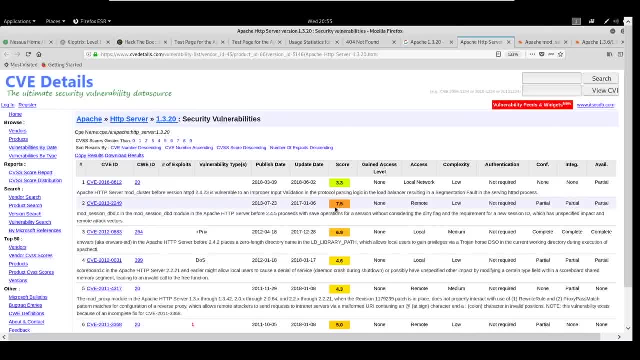 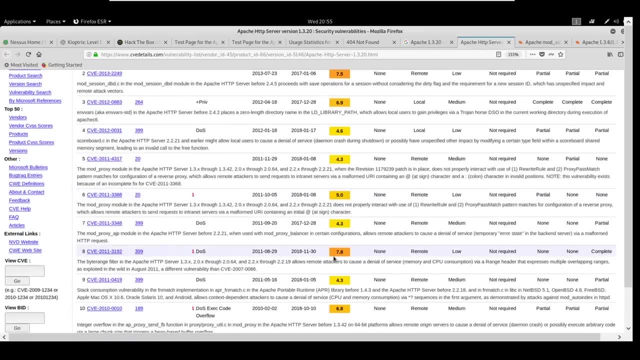 number, but basically the closer to 10 we get, the juicier. this is of an exploit and you can kind of read what they do like. this one's a 7.8. it's a denial of service attack, so not something we're going to be able to do, but we know that. 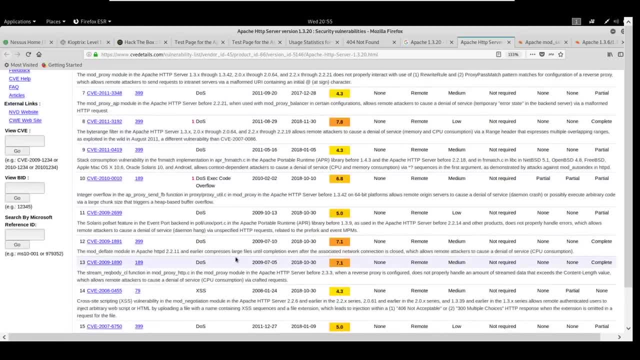 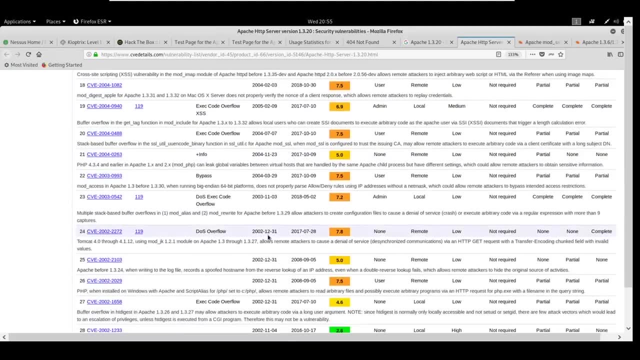 it exists same thing through a lot of these, or a lot of these are denial of service, cross-site scripting. we've seen that a few times. really, we're going to be able to do a lot of these are denial of service. we want some sort of execution like a code overflow here, any kind of remote. 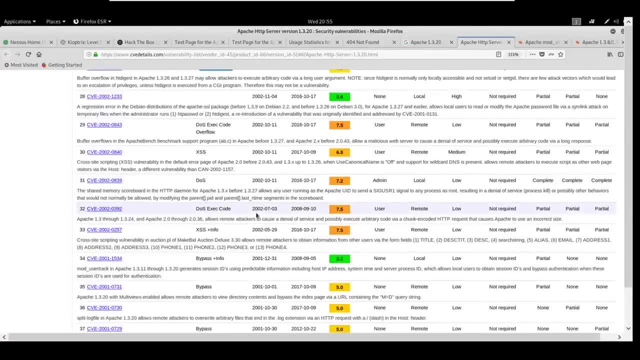 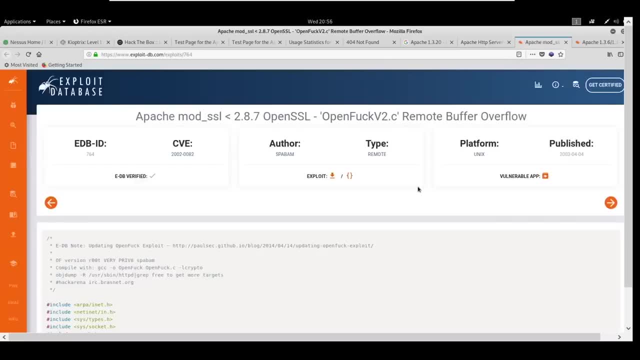 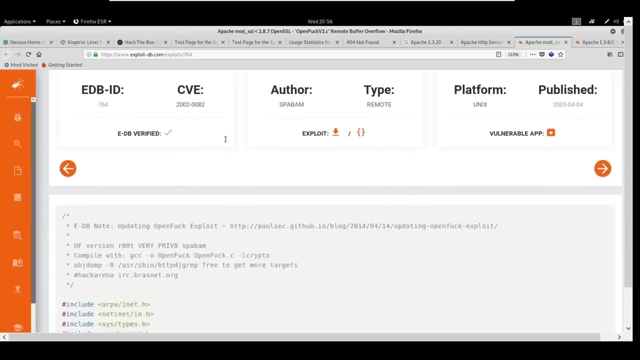 code execution that we can get would be great. so those are the types of things we want to look for also when we're on this exploit DB. let me zoom in. so this is the mod SSL 2.8.7. we would come in here and read through the code to see a. 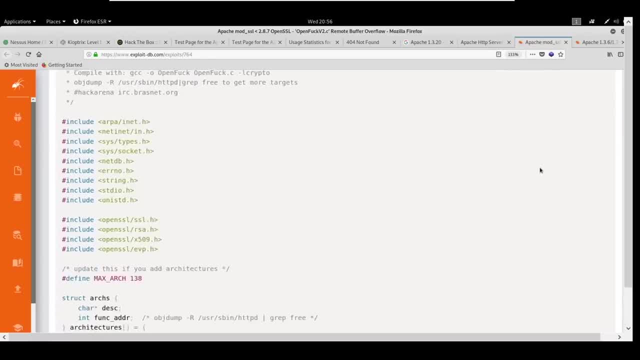 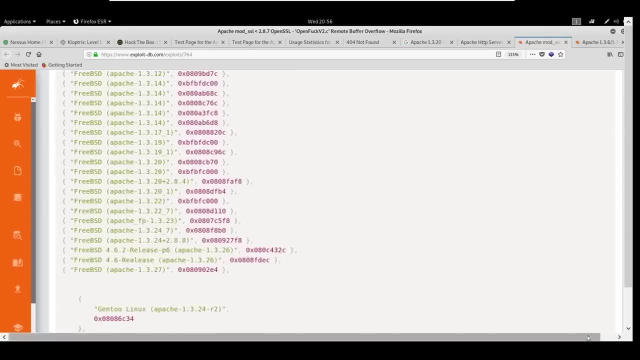 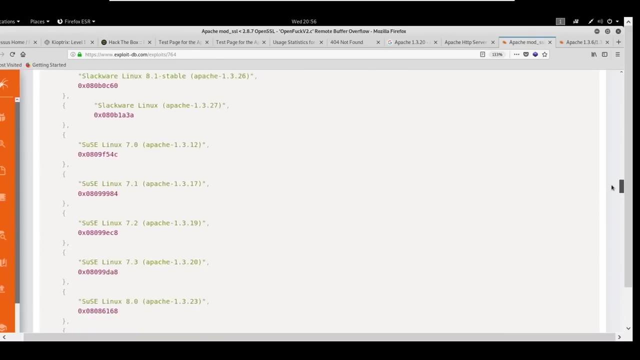 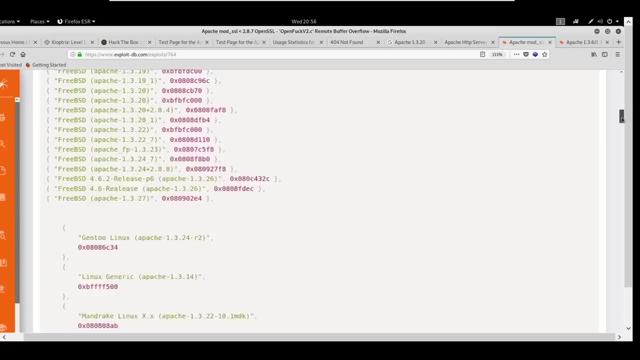 lot of times they tell you: hey, this is exactly what it affects. sometimes they just give you the code like this: let's see what we can do if we scroll down. okay, so it looks like it actually it's vulnerable- vulnerable for quite a few things. let's see if there's notes in here at all for this. so 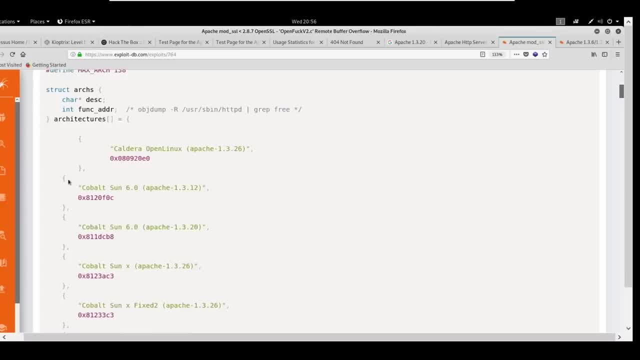 depending on the system architecture. in what's running they have different addresses. so I did see Apache 1.3.20, so it would have to line up that it's Apache 1.3.20 and we're assuming that we're running some sort of Red Hat Linux. 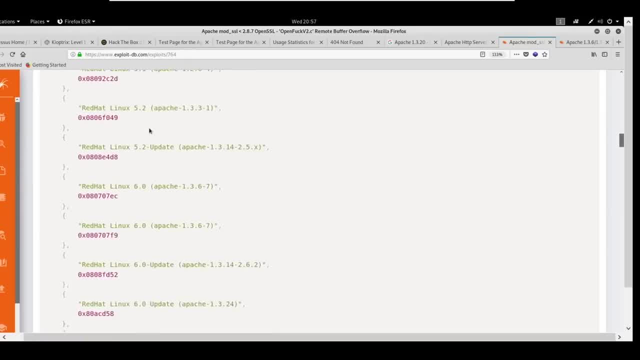 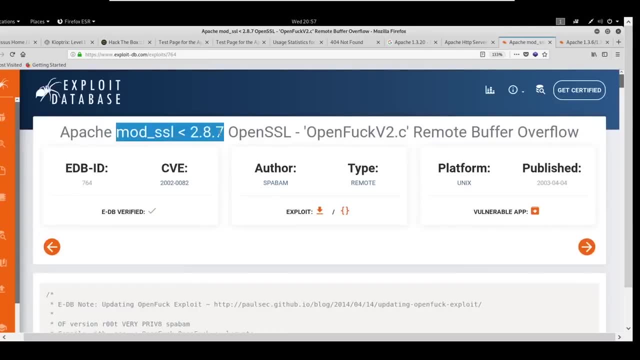 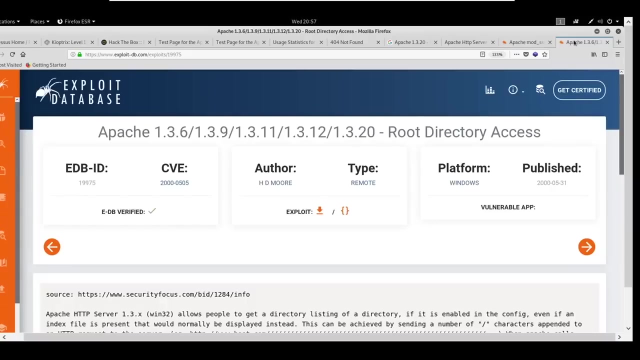 which it does have Red Hat Linux in here. so this may be something that we're interested in, especially with the fact that we have that, that mod SSL condition as well. so this is something that we would save. we would save for later, and some of you are getting a little bit ahead of me. so yeah, it is exploit city. 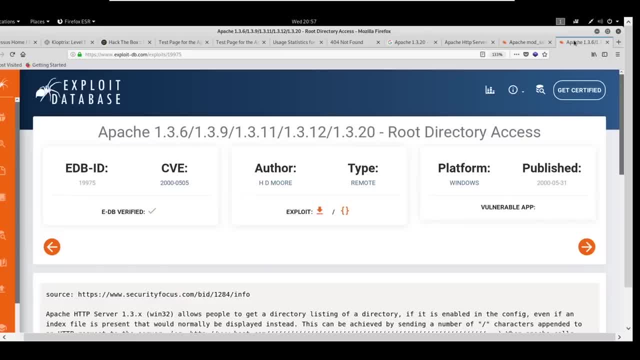 over here. there are quite a few exploits with this machine. somebody asked: do we normally see so many vulnerabilities in a website? no, we typically don't see this many vulnerabilities. this is a. this is a beginner machine built many years ago, so I I even think that there's vulnerabilities on this machine that the 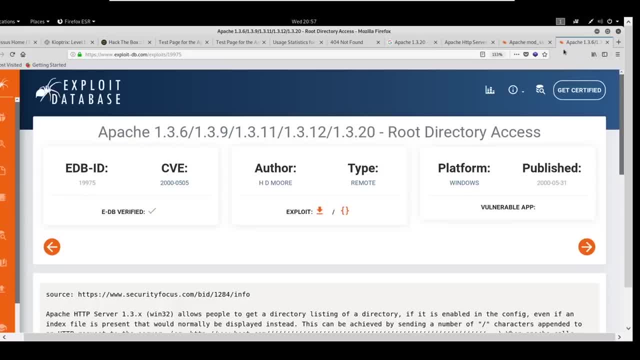 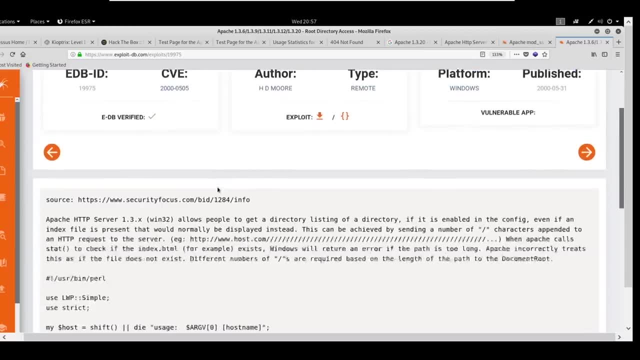 creator didn't even know existed. so I don't think that there's vulnerabilities on this machine that the creator didn't even know existed at the time. that's how old this machine is, so we can look at this as well. let's see if this one has any info on it. Apache HTTP server allows people. 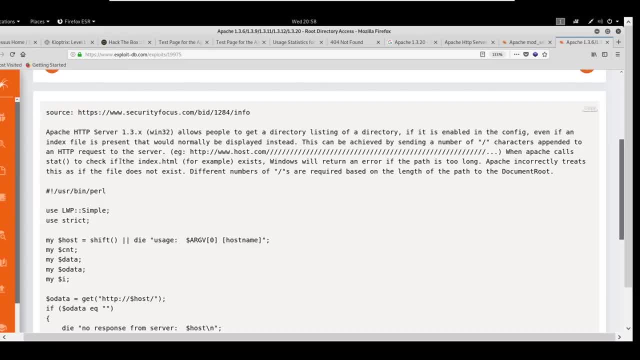 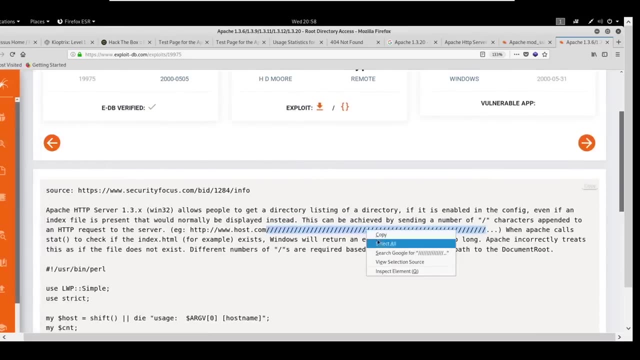 to get a directory, listing of a directory, if it's enabled in the config, if index file is present. so you saw. you saw the the many, many, many lines like that. this is looks like what was going on. we can copy this and see if this is actually there. but we saw that earlier. 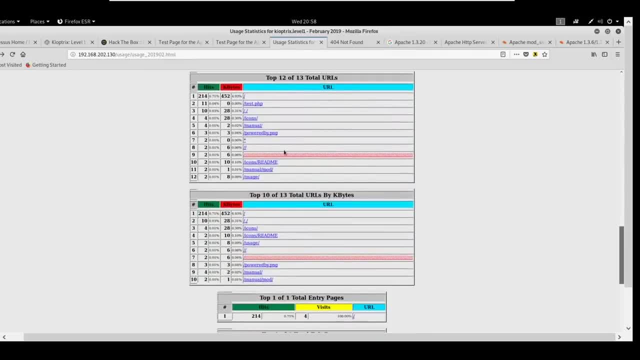 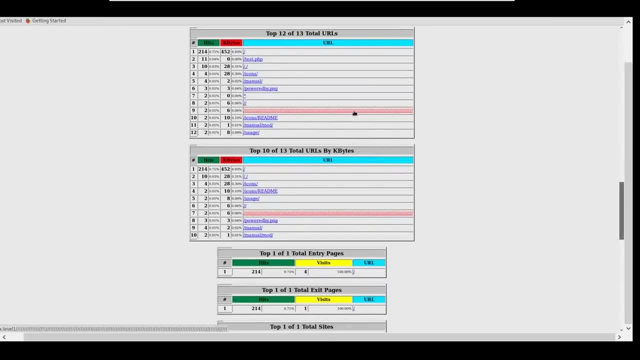 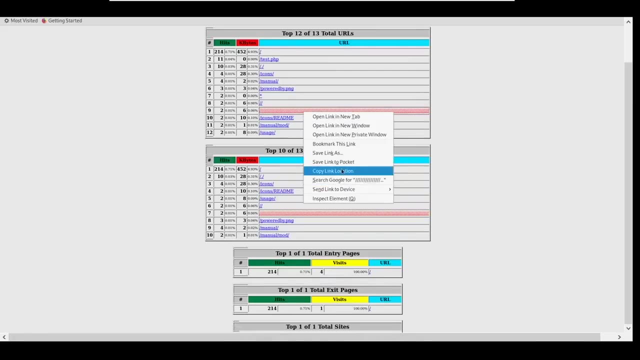 when we were looking at that statistics page, if you recall correctly, and maybe it wasn't going to that address. I'm not sure what was happening. no, oh, it's trying to. it was trying to resolve the host name is key objects, level one. so you copy link location, let's paste it and see what happens if we go back to the. 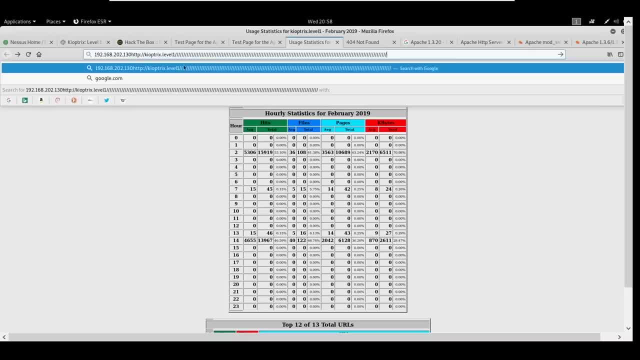 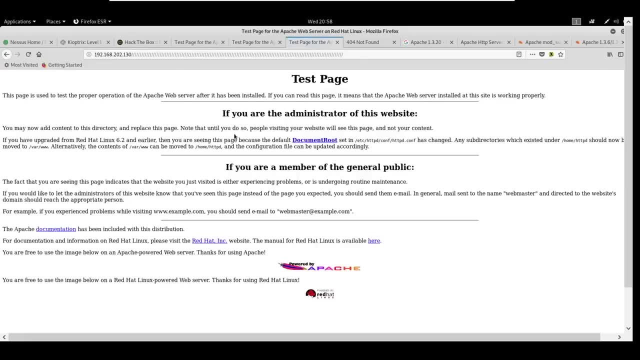 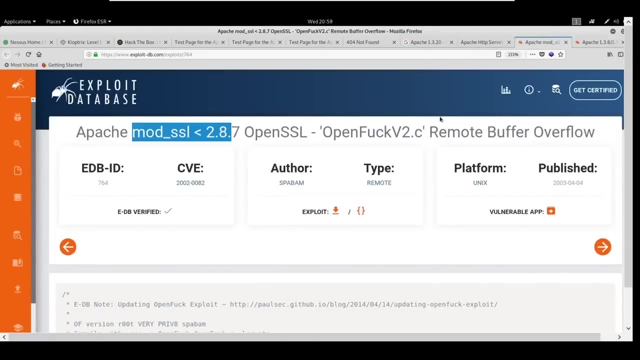 it's trying to. it was trying to resolve. the host name is key objects, level one, so it happens. get rid of some of this stuff. it just takes you to a test page. so somebody mentioned search splite. that's the next thing that we're going to cover, and since 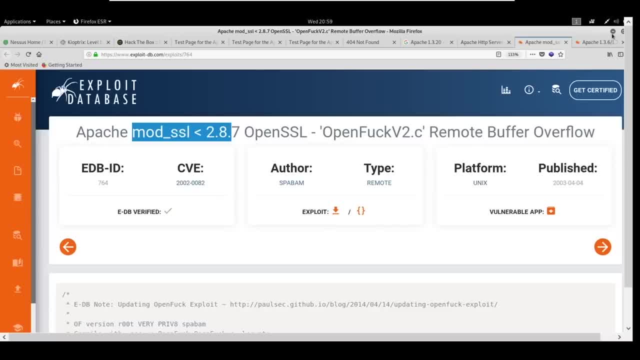 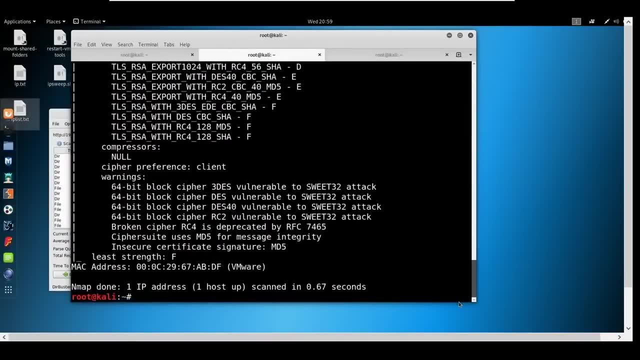 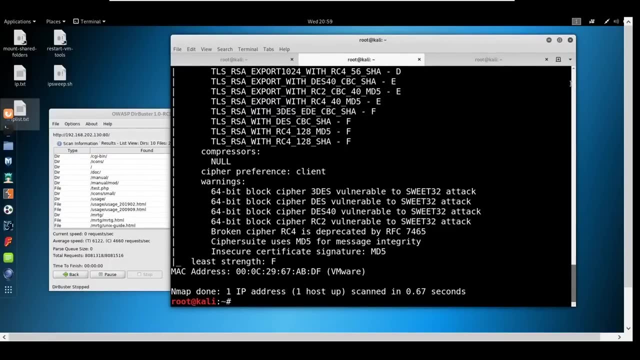 you all are asking about it. I will cover that. somebody asked what I was drinking. the answer is diet Mountain Dew. sorry, nothing fun tonight. okay, let's look at search split. so if we type in search plate, this is built in. this is just like a local repository or store of exploit DB. that's already out there. but 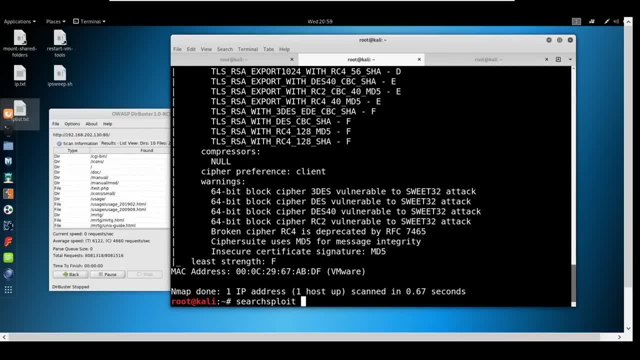 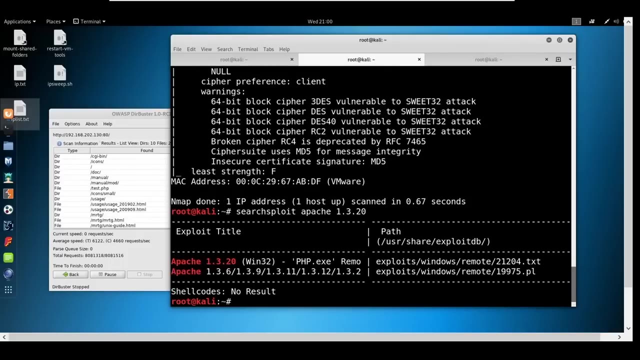 sometimes you find some, you know interesting things, or it's a quicker way, especially if you're offline, to look up some of these attacks. so I like to search it a few different ways. so say, we're looking for the Apache 1.3 point 2: 0, we could search Apache 1.3 point 2: 0 and it comes up. that is to me. 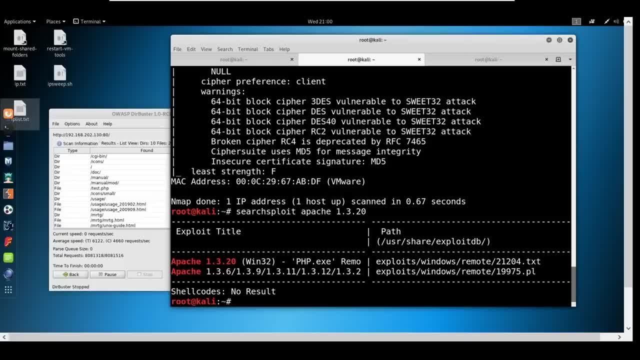 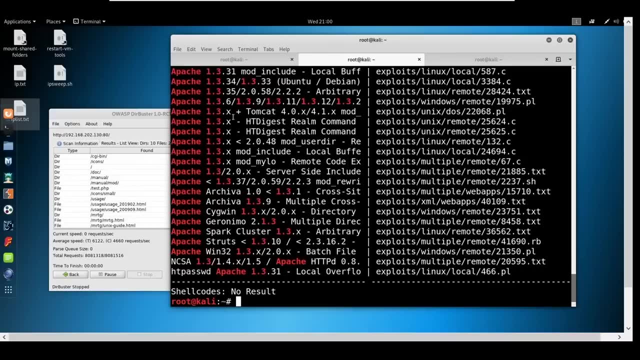 very, very surprising. it's not common that it comes up with a specific number like that. typically there are range and you lose a lot of information. I think when you search like that, I like to do one point 3, something like that, and you'll see like it has the dot X through a certain range and then you really 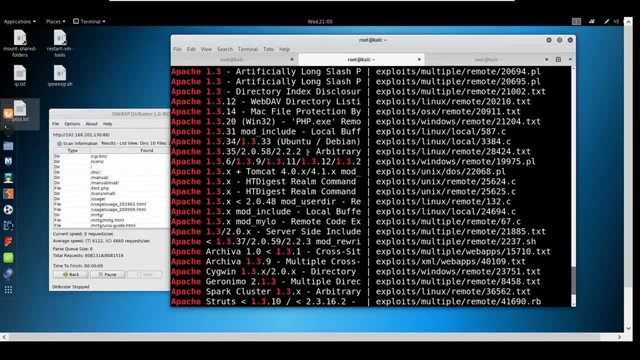 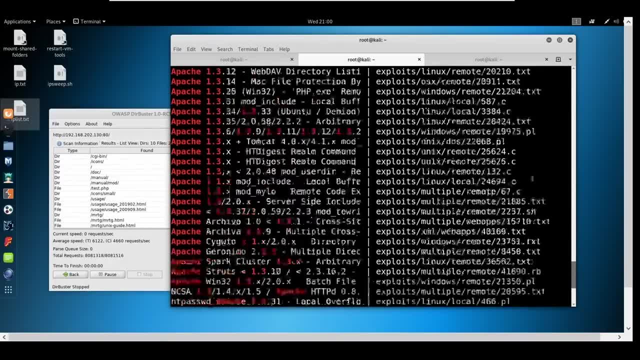 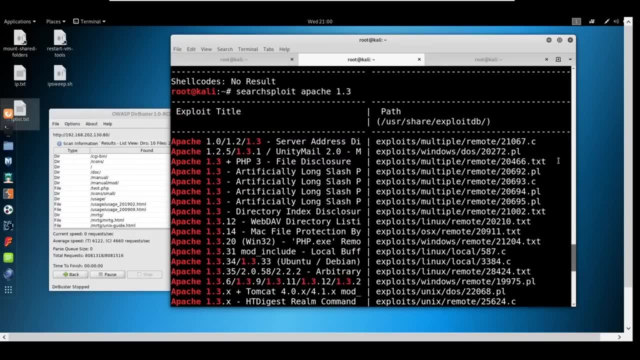 start to pull up some of this information. but let's just say we looked up 1, point 3, point 2: 0 specifically it gives us the exploits in here so you can see like a file here is in written down, written in C. This one's written in Perl, This one is a text document, So when we see it written, 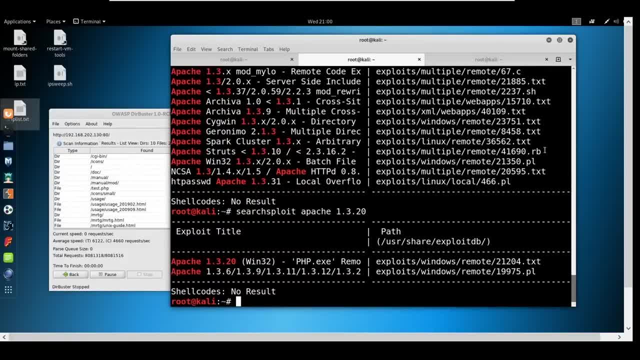 in Perl, we can assume not Perl. So if we see it written in Ruby, we can assume that it's probably part of Metasploit, because Metasploit modules are written in Ruby. But we could take a look at one of these, say Apache 1.3.20.. We could say we could just cat out that file user share. 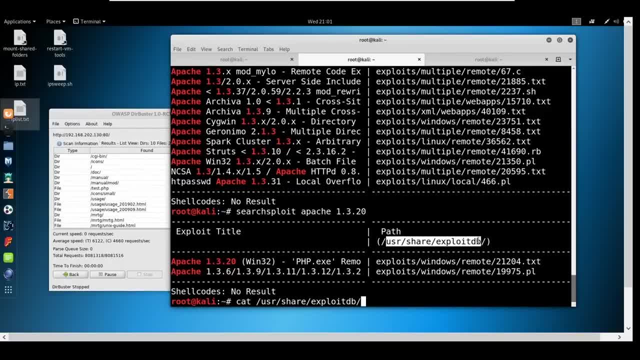 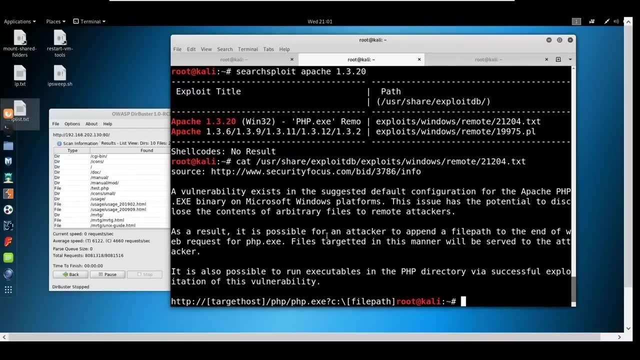 exploit DB, And I'm pulling this information from right here And then I'm pulling the rest of it from right here: Exploits Windows remote and then 2.1.2.0.4.txt, So we could see what the 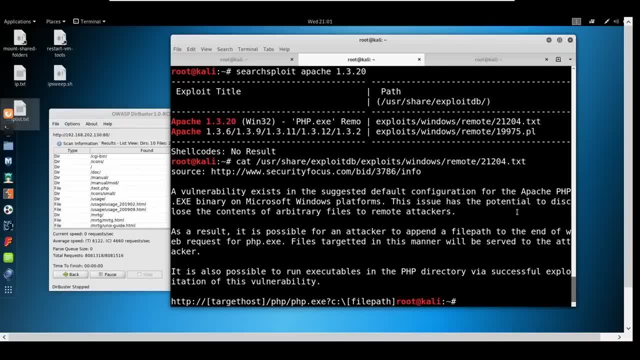 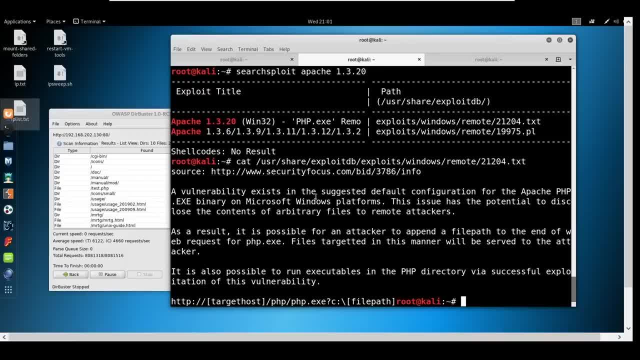 example. this is why we do our research and we see, okay, well, we know we're running an Apache server, but we know we're running on Red Hat. so when we look at an exploit like this, we know, okay, well, it says Microsoft Windows platforms. we're not gonna run this exploit anyway. so it doesn't matter and it's one that. 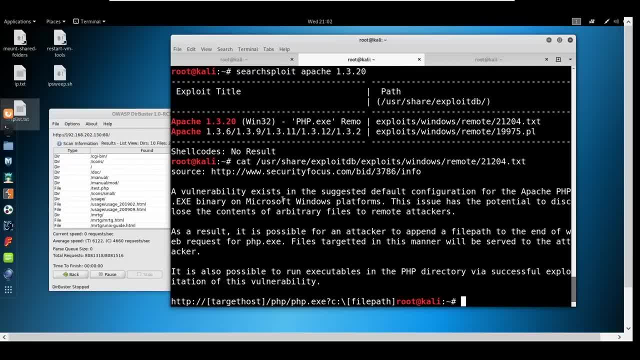 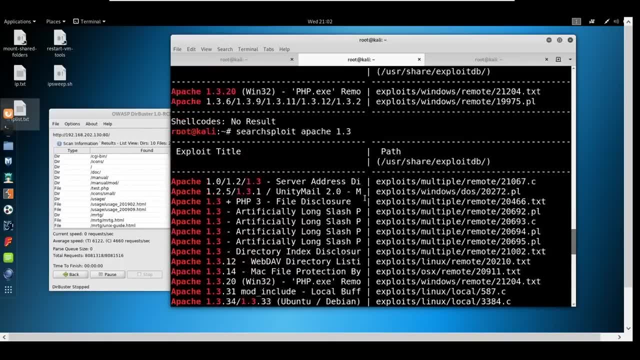 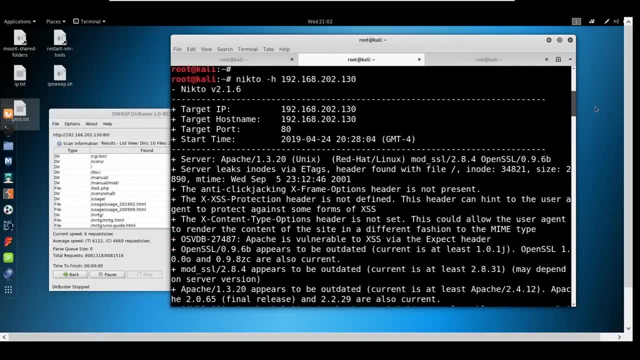 we can ignore. so some other things that we can look at. so we definitely found some interesting things with Apache. we would want to look into the mod SSL and we'd want to look into, you know, as much as we can in here. so let's see what else. 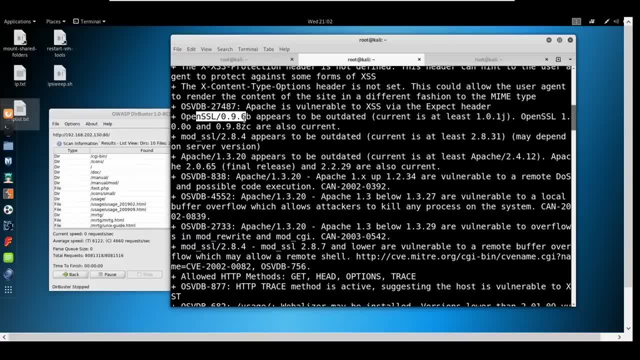 there was Apache mod SSL, open SSL here as well. so I would say this is our bingo right? this is one of the the big bingos is. we saw this come up. we saw all the conditions meet with the Red Hat: the one point. three point two: zero on the Apache, the mod SSL, two point. 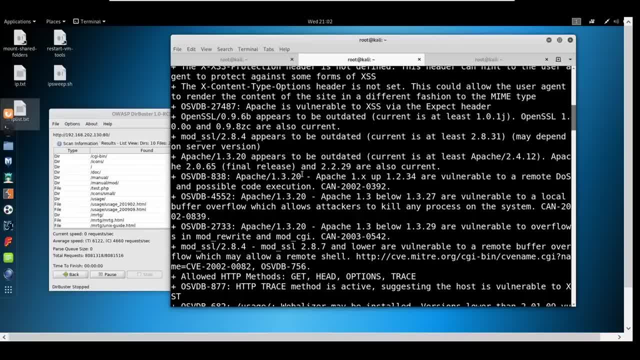 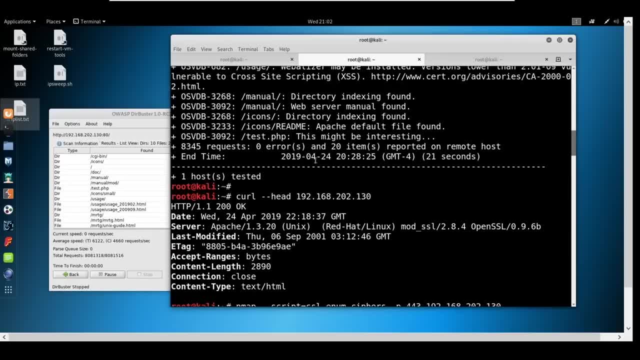 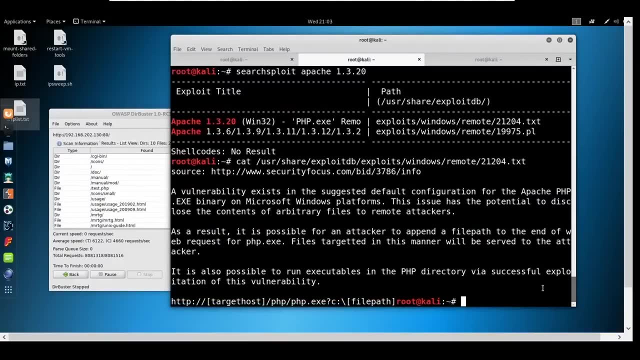 eight, point four, all really met up and worked out. so, alright, let's look up now, let's let's back away, because we've been at this for an hour. let's back away from the website just so we can see some other other things, because there was. 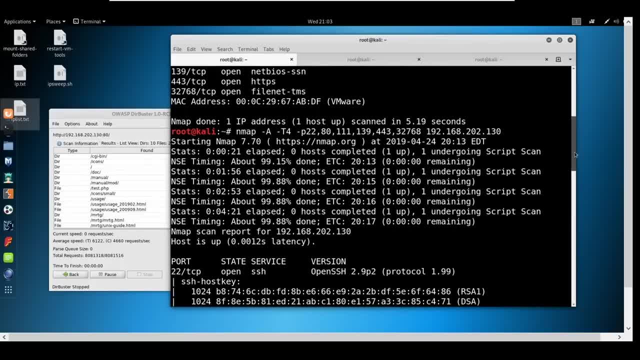 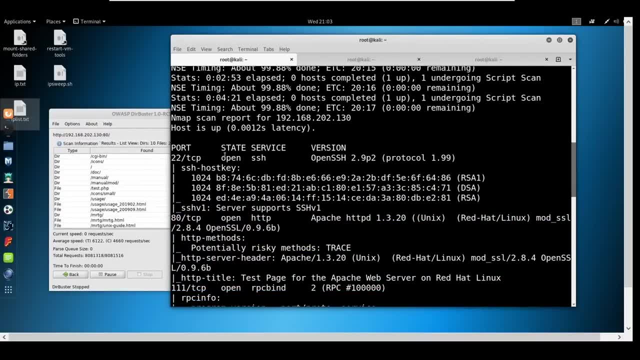 other things on the search. so same procedure, though right when we're looking up, say, port 22 for SSH. there's a couple things that I would want to try here. now there is open SSH 2.9 p2. we can search, exploit this, we can. 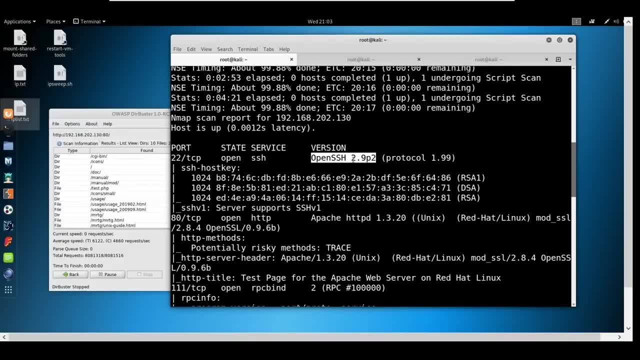 look this up, like you saw with the Apache, and we can go through and see what kind of vulnerabilities are out there for this. maybe there's something in there that gives us a remote code execution. we can get a shell on the machine. so the first thing that we do as a a pen tester is: well, I guess it's in two. 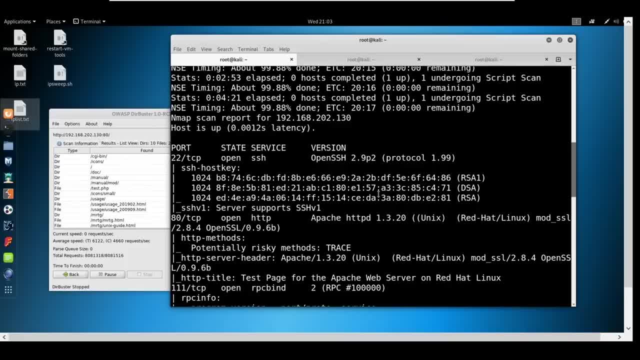 parts or two reasonings behind it. at some point we're gonna brute force this SSH. even if we get remote code execution- we get, we get all the wins we want- we still want to attack this SSH. so for the reason that we are trying to, you know, 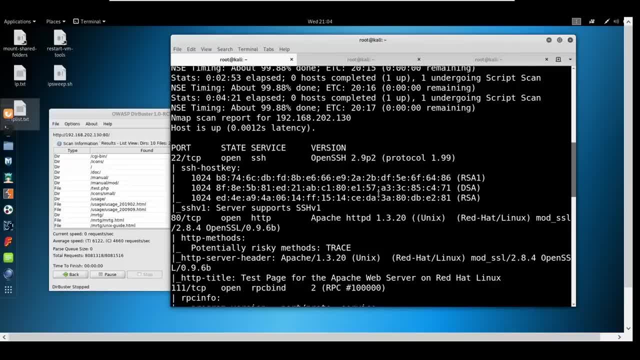 try to use the TS again. we could easily use it to do that, but we could something here before we start doing such a simple attack. they call this brute-force attack. so if we, if we attack their SSH and do a brute force attack, we want to make sure that their SIM is seeing this brute force attack. if their 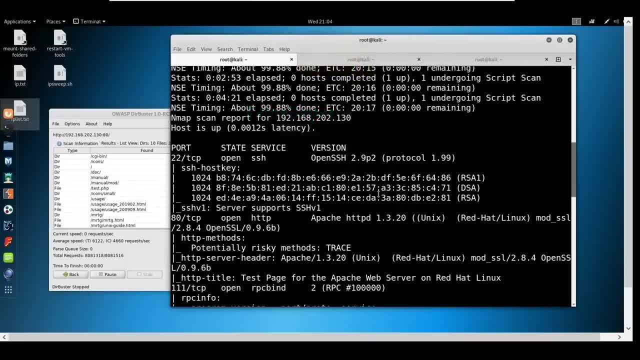 SIM is not seeing the brute force attack. we're running this attack and they're not catching us. that's bad right. another reason here. let's say that we don't have anything. but let's say that we've gathered some usernames and we want to course the SSH with the usernames we gathered and do password spraying, which we'll talk about. 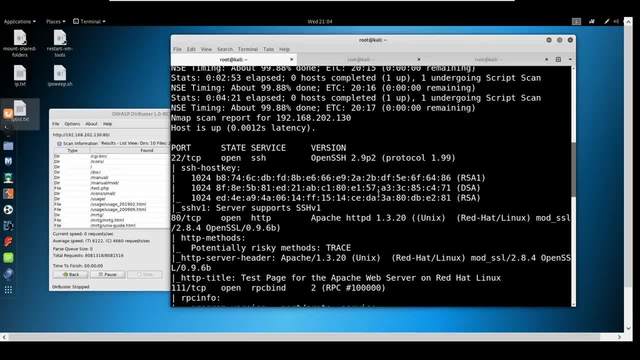 when we get more into exploiting and in hopes of getting some sort of user account on this machine. So it does serve us two purposes. We want to see if we can get in. I guess more than two. we want to see if we can get in this method. We want to see if we can get in this method. 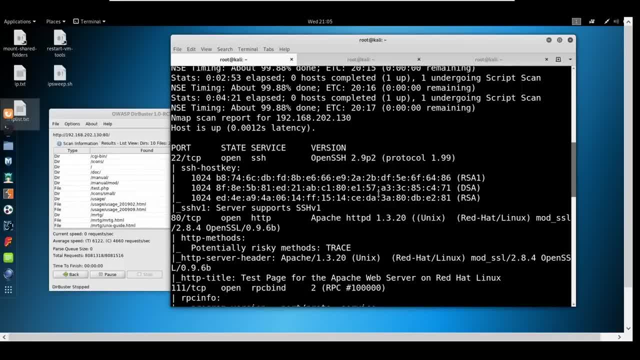 Um, is it because they have a weak password policy? Is it um poor user training? Do we find a password that's online? Is it poor password rotation? Um, those are sorts of things to think about, And, of course, we're testing their blue team to see how effective they are at. 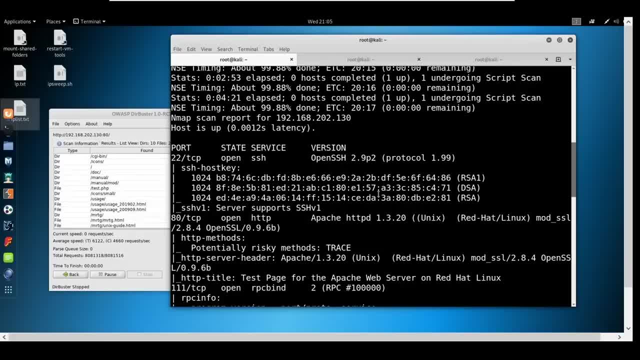 catching us when scanning. So, as we are, are doing these things as a pen tester now, not as a red teamer. as a pen tester, we are being very, very noisy. very intentionally, We want to make sure that we are- uh, we're happy when we're caught because at least they're. 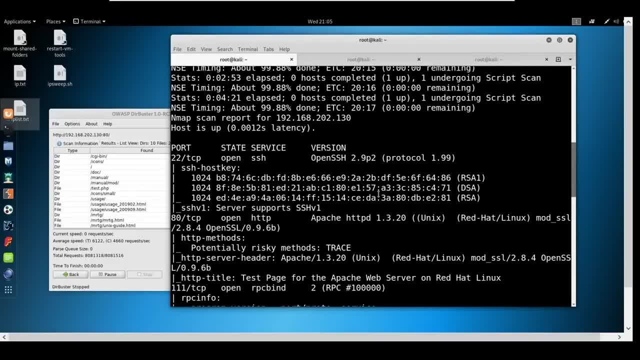 they're catching us on the basics, right, The scanning um and the, the SSH. Now I've had more in-depth where they say, okay, we've caught you doing that, Can you go back and be more quiet? Uh, we want to see at what level we see you and what level we don't see you. And that starts to. 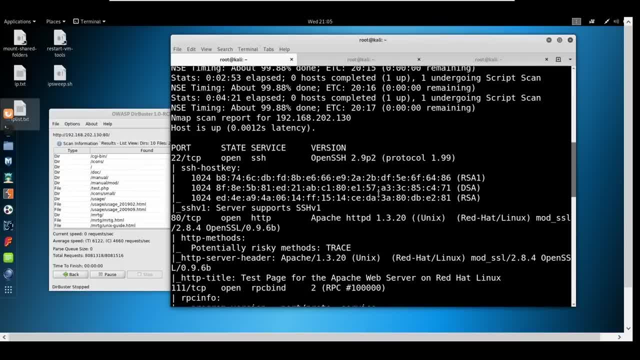 become something called purple teaming, where you work with the blue team and you try to, uh, really fine tune their SIM. But these are things that I would do on an SSH. I would, I'd brute force it, We'd we'd have to for all the reasons stated. 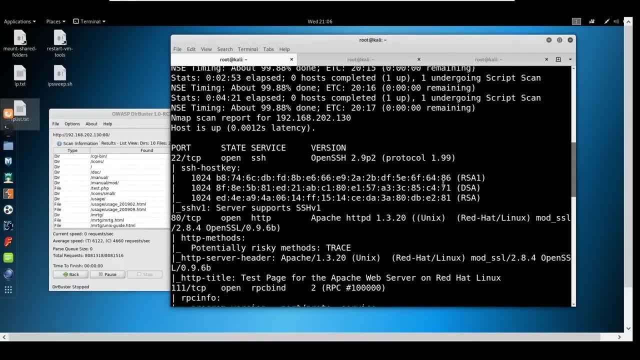 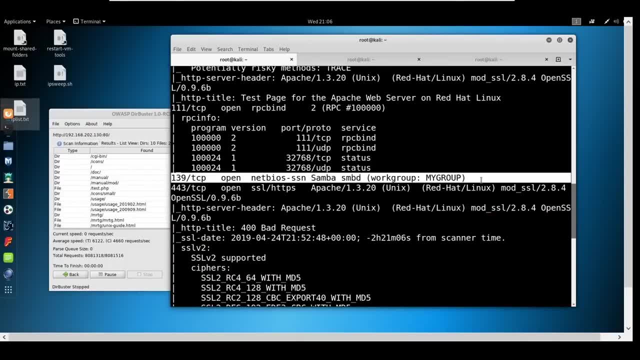 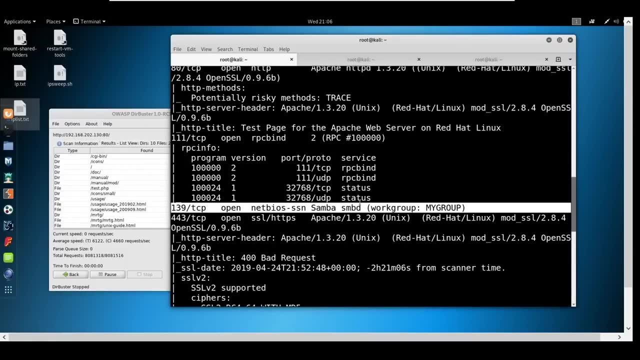 above. We're not going to do that tonight. That falls under exploiting. But the other big, big one that's out here is this 139.. Uh, we don't see 445.. Typically that's on windows machines, but 139 is our Samba share, our SMB. There are so many exploits for SMB Um. 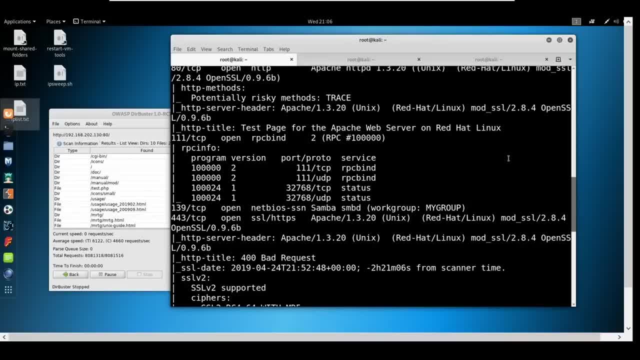 most recently, windows had the eternal blue. That's the big, big one. but you'll come to find over and over again. uh, especially as you study, like the older hacking methodologies, the SMB gets uh banged up quite a bit. So we want to look at this and just see what we can find here And SS. 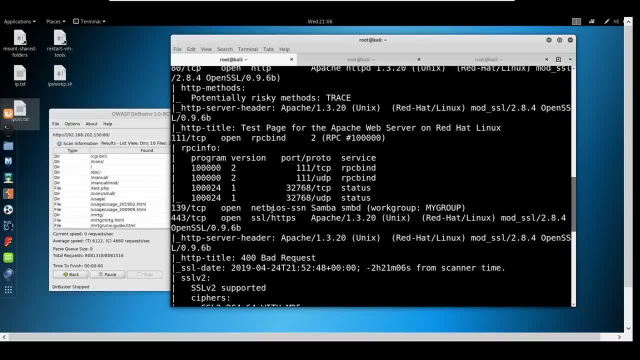 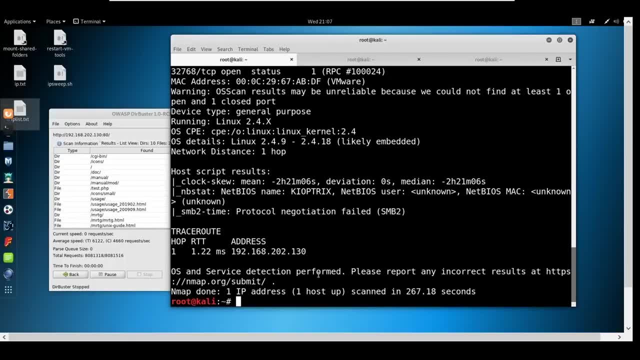 or SMB is, is always a good method for us, especially in internals, for navigating around and getting um, getting shells and gaining win. So but we'll talk about that when we get into internal and active directory environments. So when we want to enumerate uh, SMB, the first thing I do is I look at 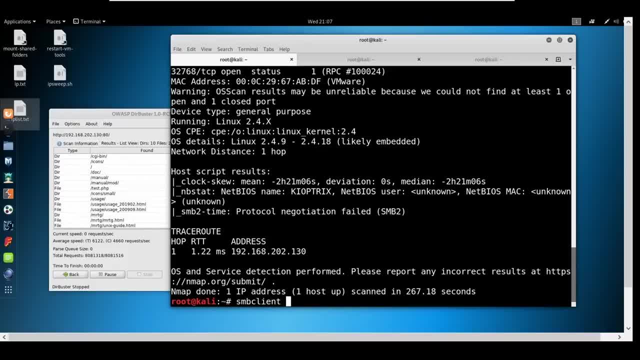 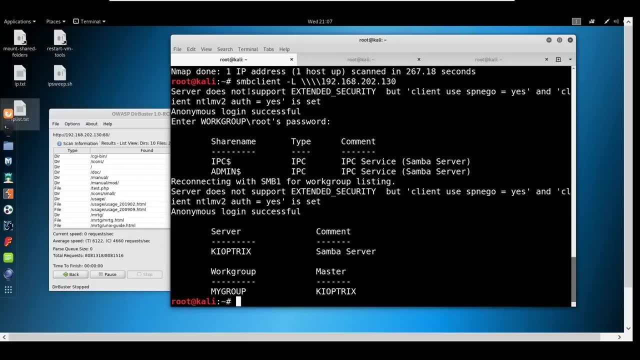 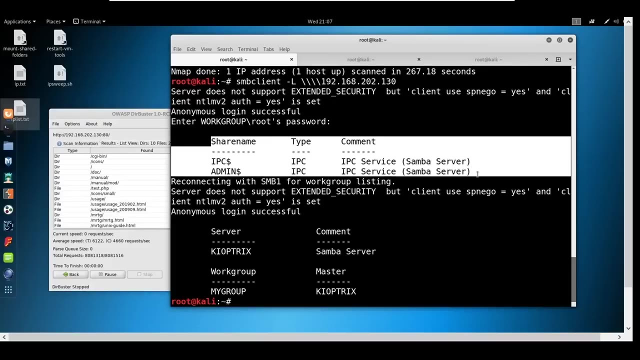 I say SMB client and I just want to do a listing And this is the format that it would be in. So it's a little bit weird due to the escaping, I believe. So I can enter in anonymous login and hit enter on it, uh, on the root password, And I can see all the file shares that are. 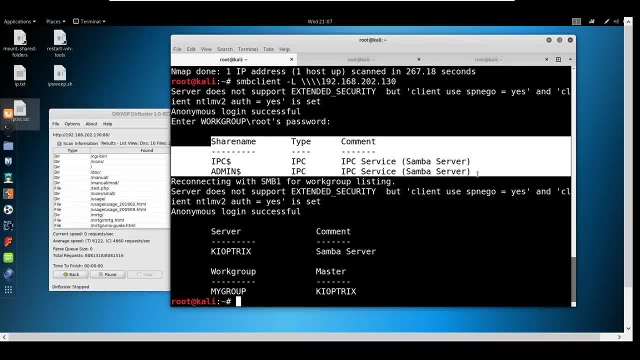 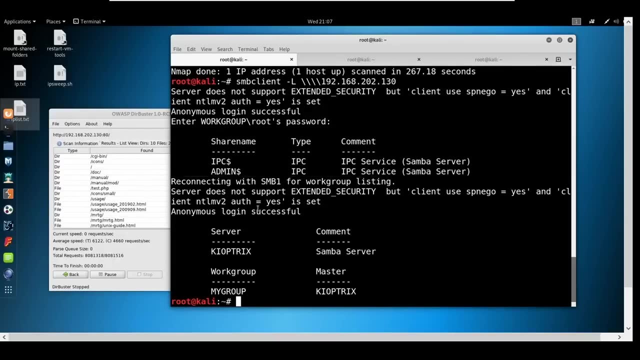 existing here. Now, this is a finding. Uh, somebody asked: should we stop using windows server as a file server for SMB? Uh, no, you just need to be uh careful with your policy. Policy is more important than anything else. SMB is just a way that we navigate. 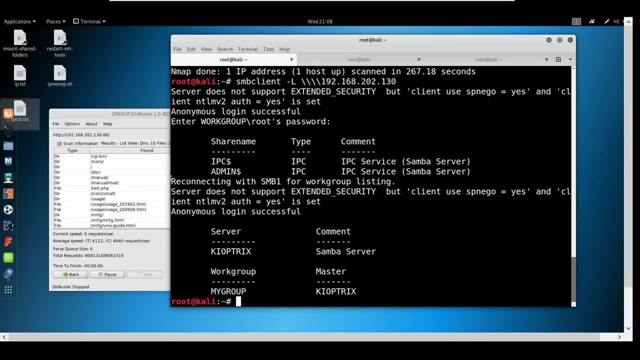 As long as you're patching um things like eternal blue, that's not the big issue. But if we're, if we're cracking passwords- and when we get into that, we'll get into it. But if we're cracking passwords and able to uh get system shells via SMB, then you're going to have 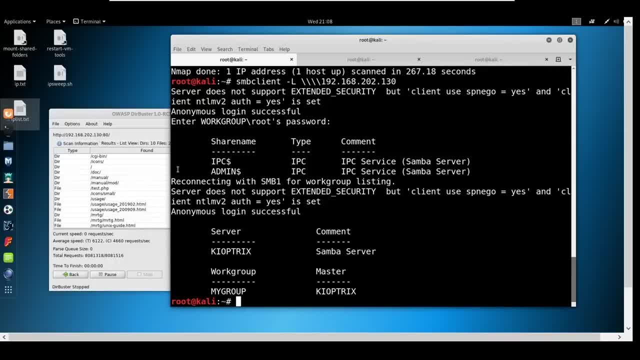 an issue because there's other underlying issues, So it's just one part of the problem. Uh, but it's. it's a way that we commonly, as a pen tester, navigate around systems, All right, So we have anonymous login here. We're able to see share names. That is a finding in. 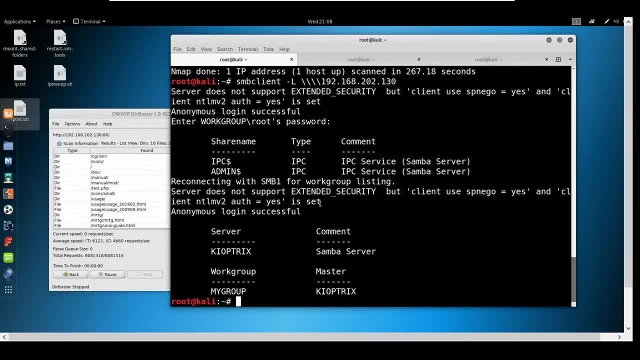 itself, because we're running kind of short on time. I'm not going to notate every single one of these. If you're still taking pictures and following along, great, Um, I hope you got an idea for how I take notes and how I would screenshot things. Um, so we have a finding. 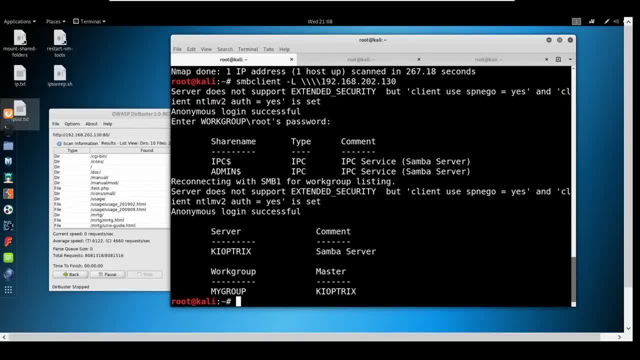 here We could try to connect to one of these- um, these shares. We could see how far this finding goes. So if we tab up and we'll say admin dollar sign, let's just try to connect to the admin and we'll take this uh dash L off. So anonymous login. 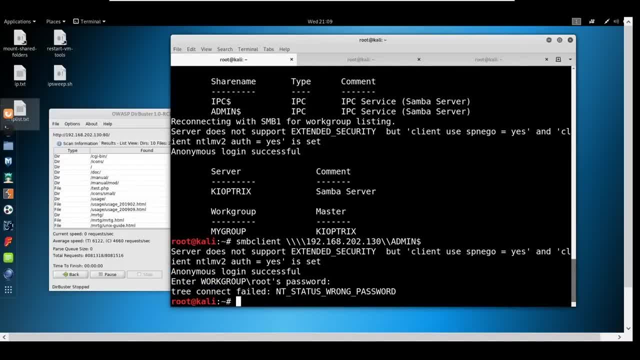 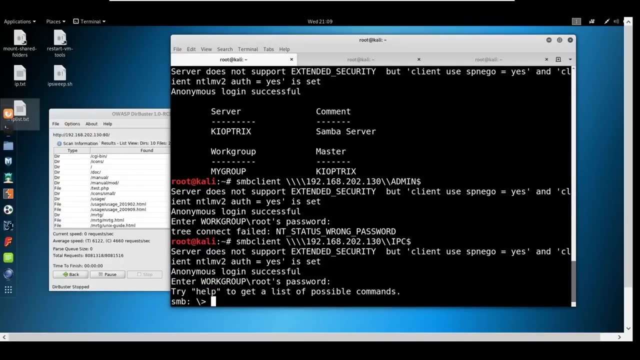 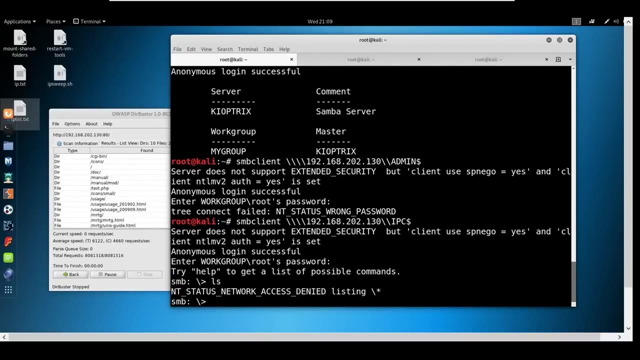 successful, We'll hit enter and it'll say: wrong password. So at least we don't have access to the admin. Uh, we could try the same thing with the IPC. Okay, We do get into the IPC With an anonymous login. we can LS in here and we're denied listing on this. Uh, we just type. 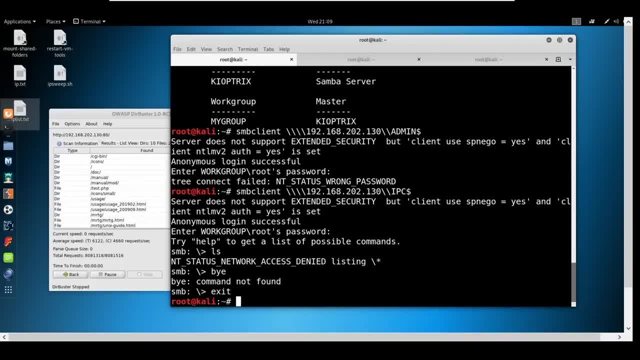 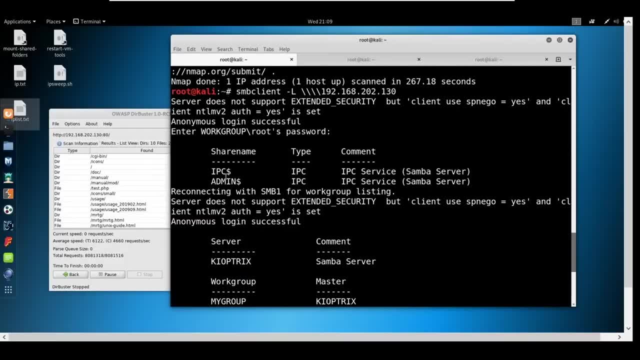 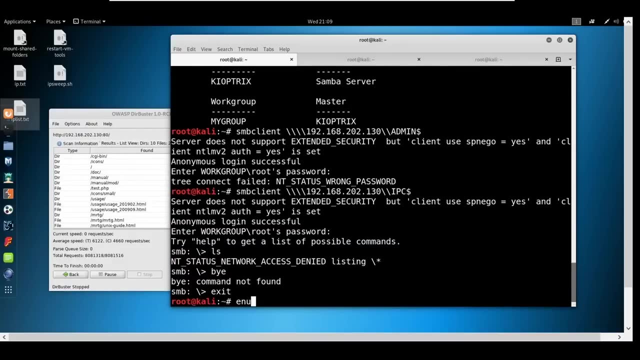 exit so we can navigate around. Um, if that opportunity was there for us. but we do have shares that we're able to see, which we shouldn't be able to as an anonymous user. Uh, there was a good tool back in the day that no longer works. It was called a new. I don't even know if it's. 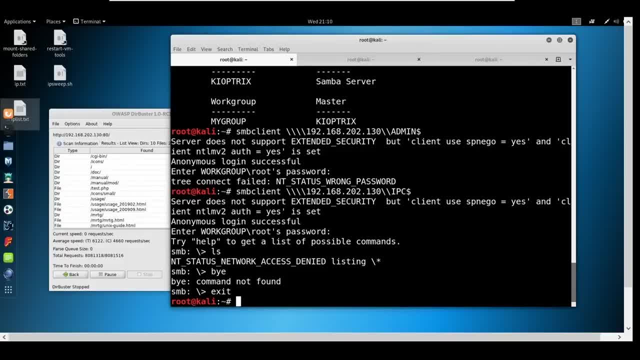 on here anymore. Nope, It's not a new for Linux and it does not. uh, it does not work anymore. It's not around anymore. I don't know if it just stopped getting updated or what happened, Um, but uh, other people are saying they use it. I've found that it's broken with. 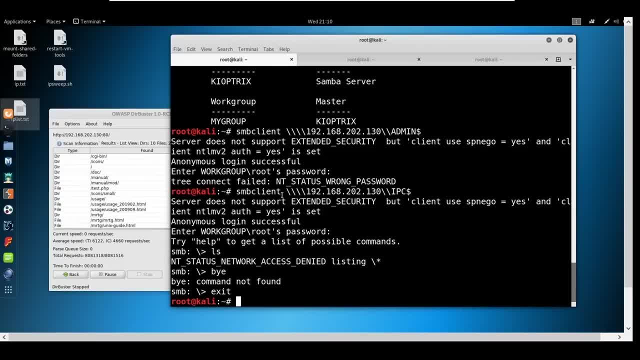 more recent versions of Cali and I like to stay up to date. So, anyway, it's broken with updated SMB client. There you go. So one thing I like to do is I like to find out what type of SMB uh we're running and that may have come out in the Nessus scan If we come into 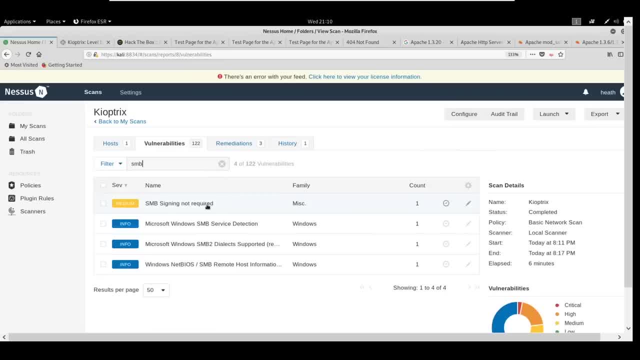 here: uh, if we type in SMB, uh, this is going to be another finding, but we'll talk about this more. when we get into internals, This SMB sign-in is going to be another finding. So we're going to talk about this more. when we get into internals, This SMB sign-in is going to be another finding. 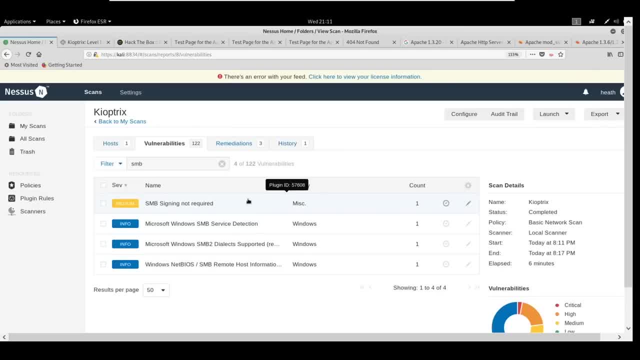 This SMB sign-in is going to be another finding. Uh, this is one that you need to have on in your active directory environments especially. or else we can just relay credentials without ever knowing the password and gain um shell access to a machine. 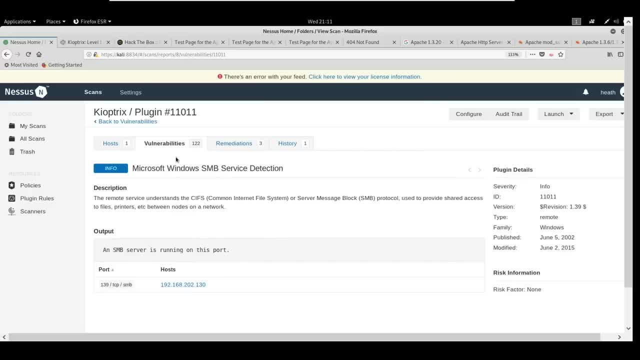 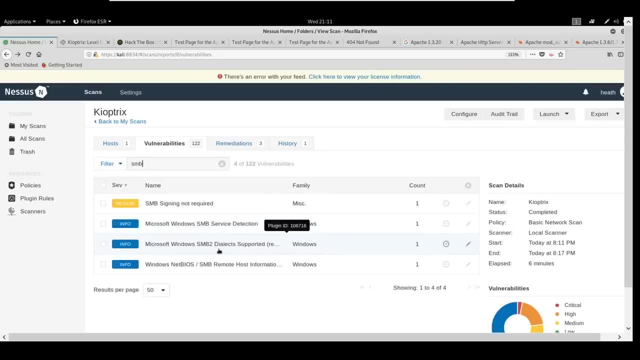 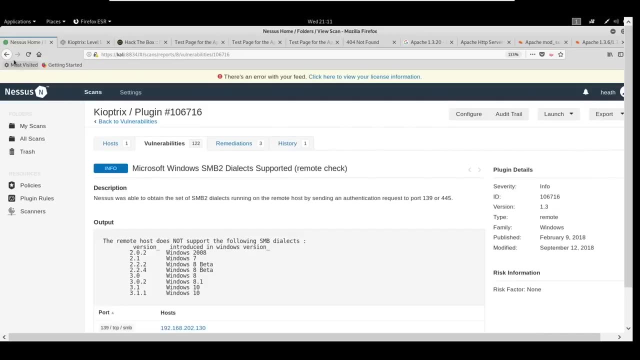 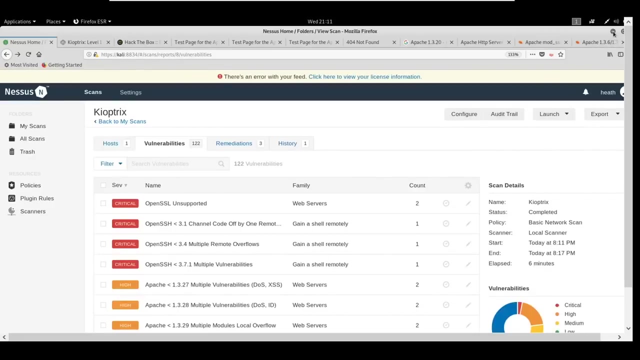 So we've got service detection doesn't specify the SMB. Let me look at the other two. real quick Dialect: supported remote host information. Let's see- Uh, I don't think it's an actually tell us. All right, So what we're going to do is we're going to use Metasploit. 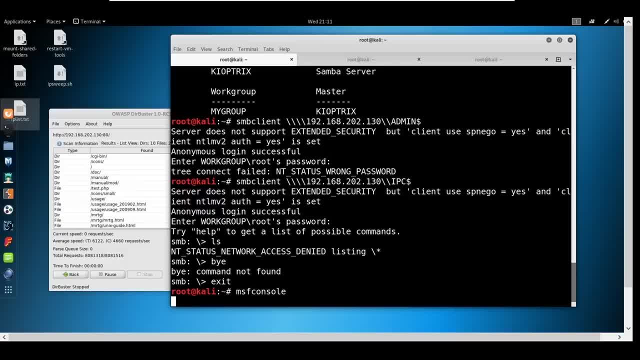 So we're going to type in MSF console and we covered this last time, Remember, we talked about the different features. We talked about auxiliary and export and export. So we're going to type in MSF console and we covered this last time. 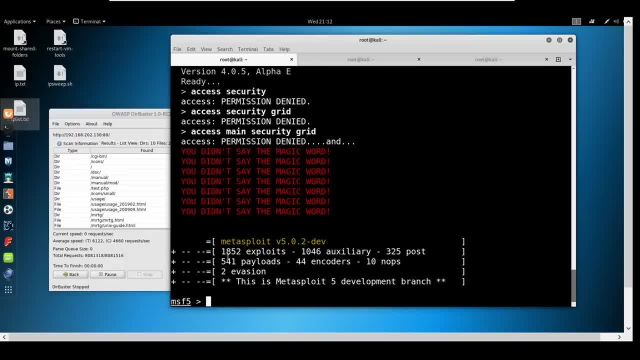 So we're going to type in MSF console and we covered this last time. So we're going to type in MSF console and we covered this last time. Um, and if you look here actually has the, the exploits, auxiliary post payloads, um, actual, 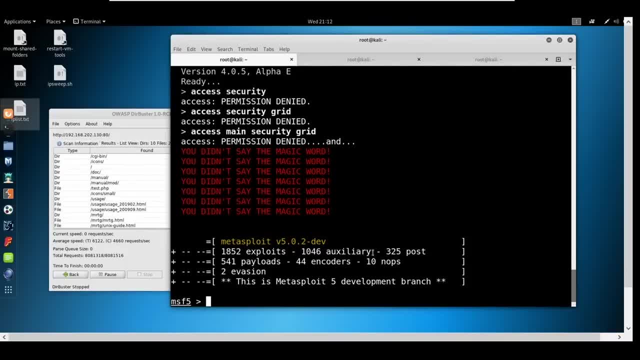 payloads, encoders, et cetera. Um, we're typically going to live in these three. We'll use this one. if we're doing some sort of um, well, we'll, we'll use these as well. Uh, so, but we're going. 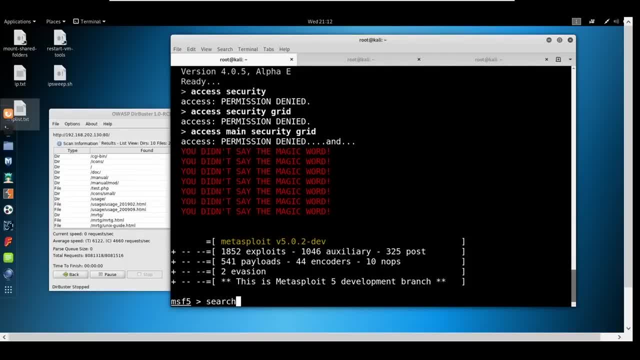 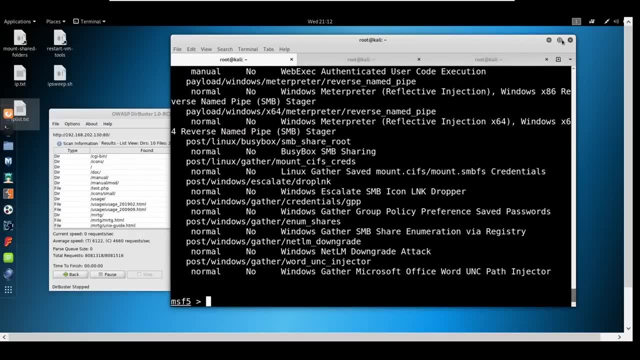 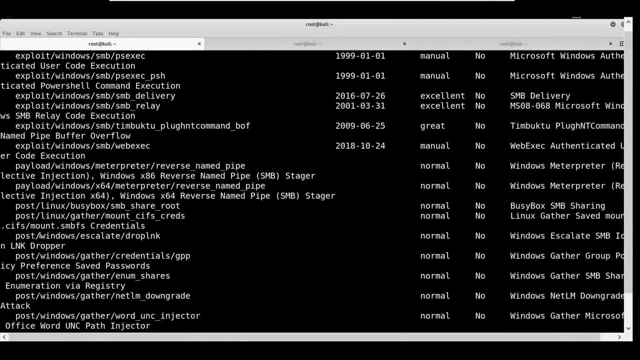 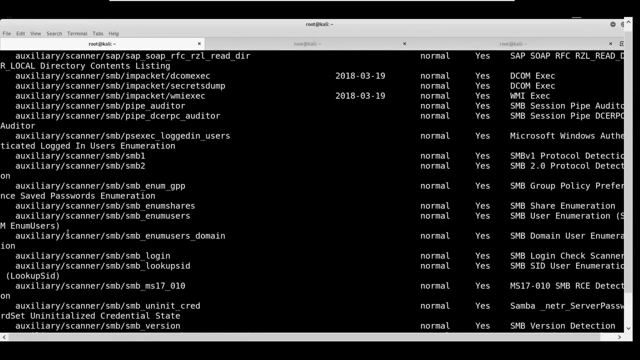 to be focused on auxiliary. What we're going to do is just for fun. we're going to search SMB And there's a lot of information here. So even if I scroll down, it kind of organizes it by auxiliary exploit then post. post means once we've exploited a machine, exploit is an exploit We're looking for. 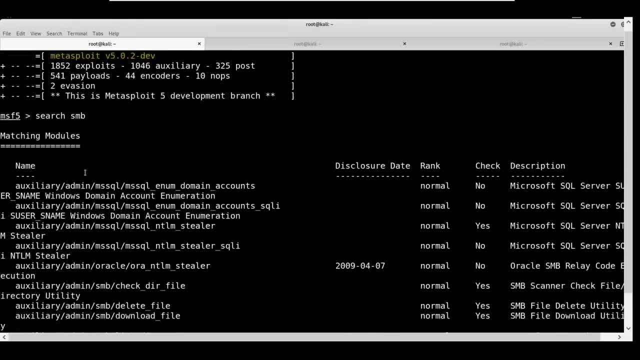 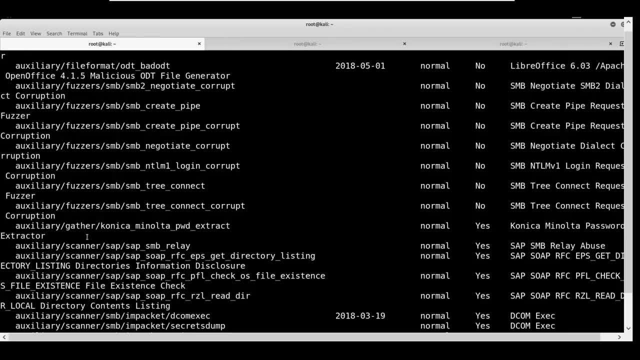 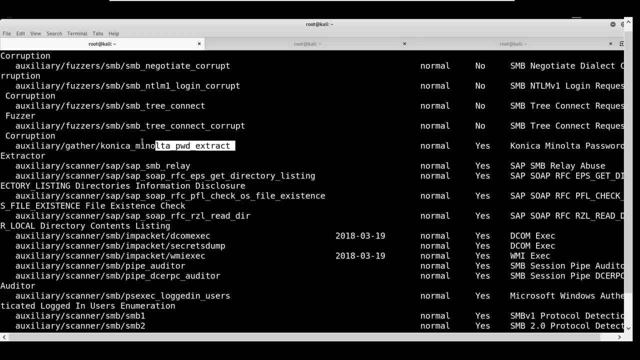 an auxiliary scanner. I'm going to scroll up to show you all the different ones. There's auxiliary admin. there's auxiliary dial service. uh, fuzzers gather. Oh, I have gotten a. I've gotten active directory or domain admin off of this guy. 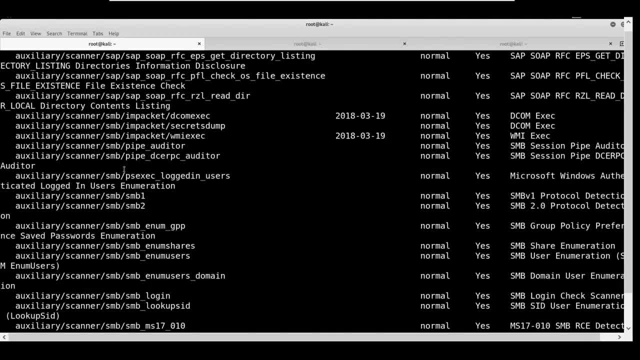 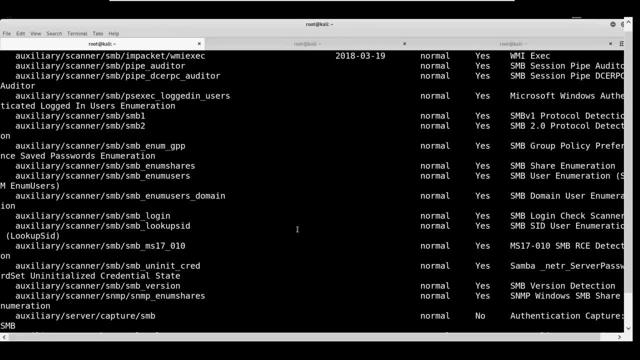 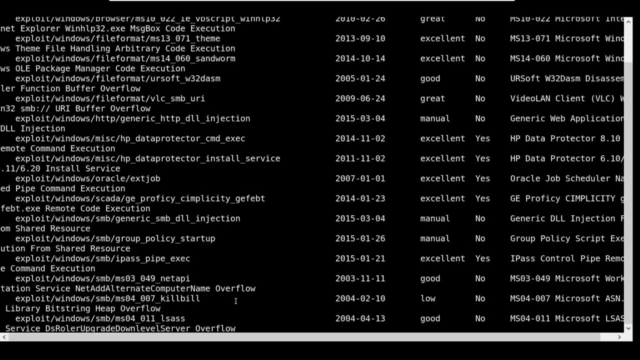 believe it or not? Uh, okay, So we're going to be using SMB version. So this guy right here, auxiliary scanner SMB, SMB version. So we're just going to say use and then you can just paste that in. 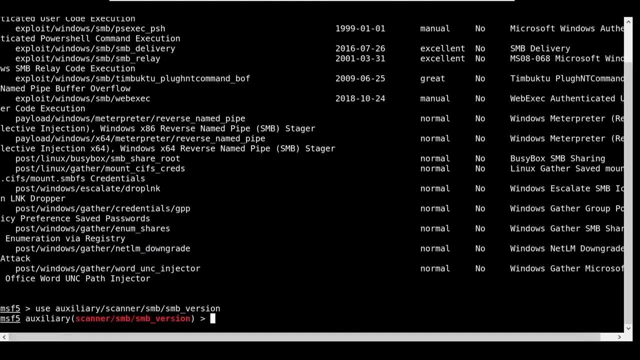 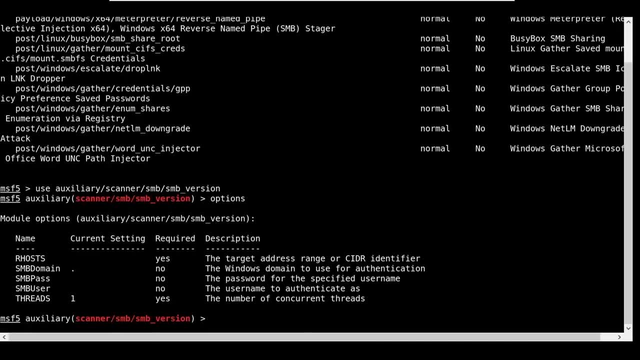 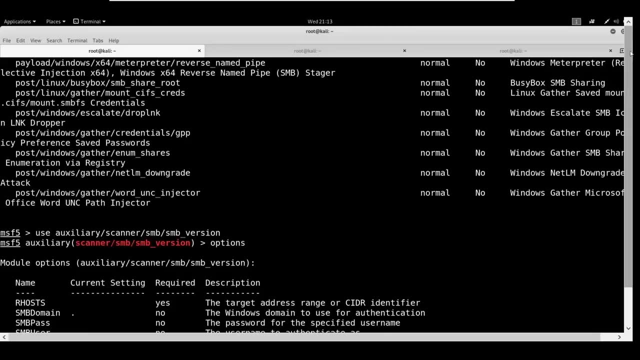 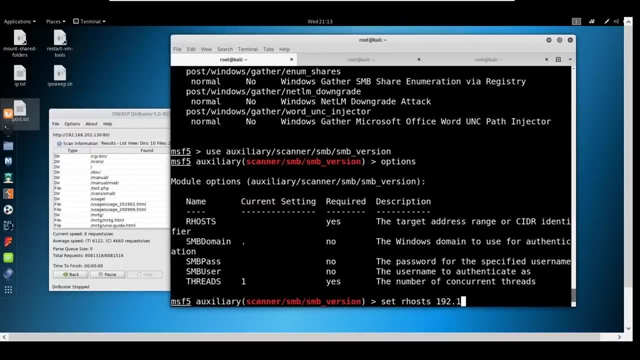 And we're going to say options, set our hosts, And then again I am a terrible person and have forgotten the IP address of this machine. It is 1 9, 2, 1, 6, 8, 2, 0, 2, 1, 30.. 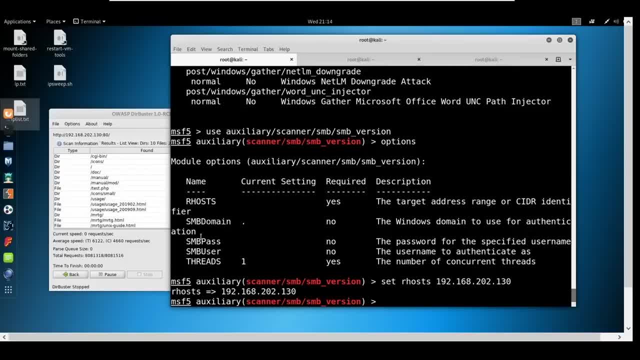 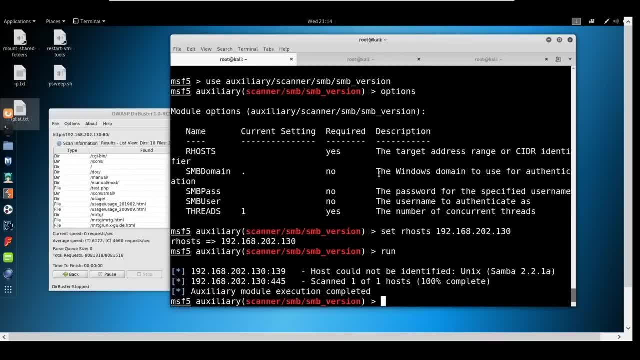 Okay, And we don't have a domain that we're on, So we don't need to set that. We don't need to supply a user or password because we don't have it And we'll just hit run Okay. So it identified it as Samba 2.2.1a And somebody asked: are we going to solve a? 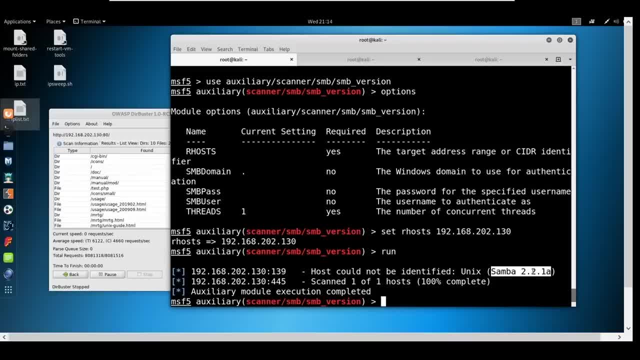 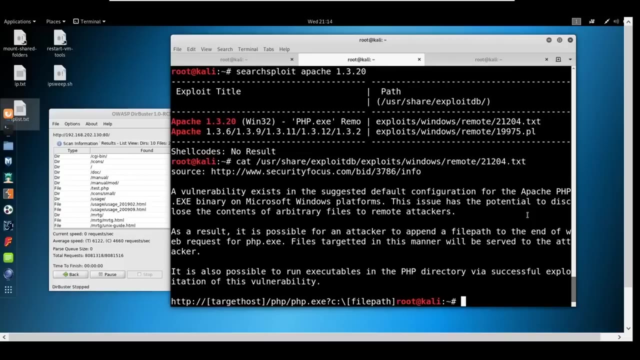 hack the box machine after this. That is not the intention. Uh, the intention is to enumerate a hack the box machine after this: Uh, we're not going to be solving, because solving requires exploitation And this week is not on exploitation. Okay, So we've got Samba 2.2.1a, We're going to copy this and let's just do search, exploit and 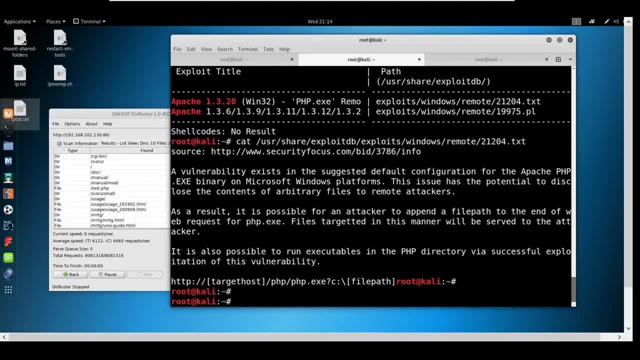 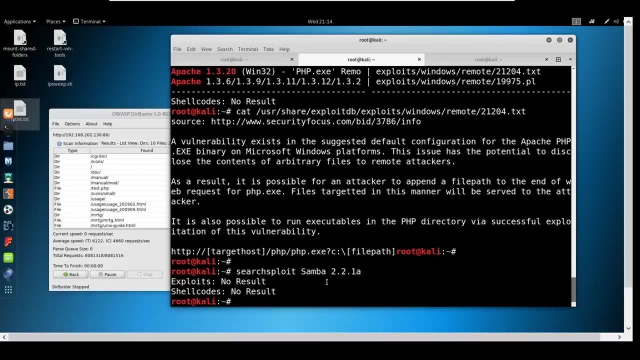 see what kind of information we can find Now again: um, um, uh, uh, uh, uh, uh, uh, uh, or may not find something with it. when you just type it out like that, No result. I like to do: 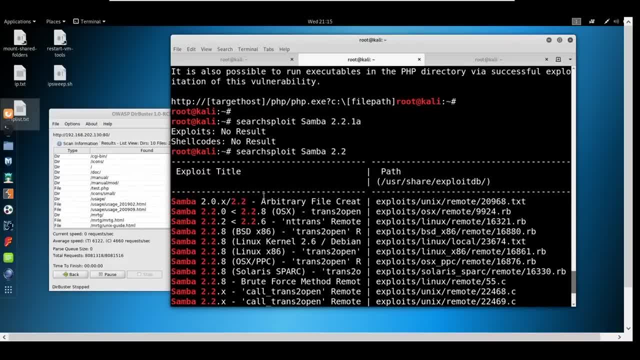 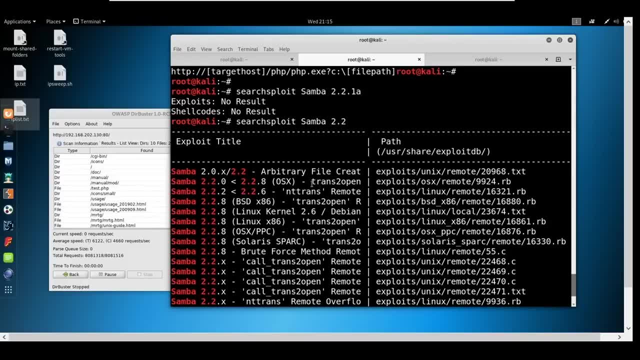 2.2, something like that. You don't make it too specific again and you may be able to find something. So it looks like there is a 2.0.x to 2.2.. That's not going to work, This 2.2.0 to 2.2.8. 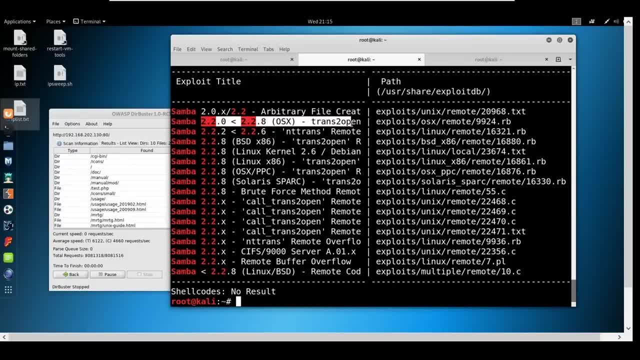 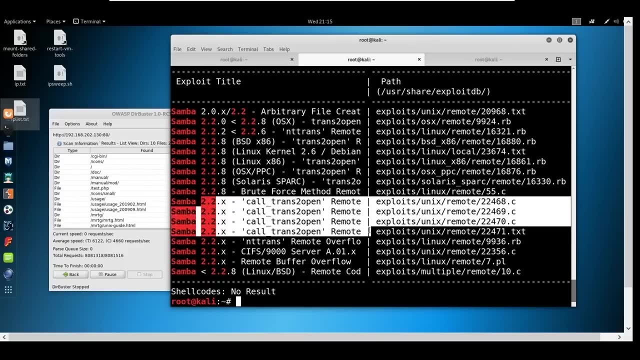 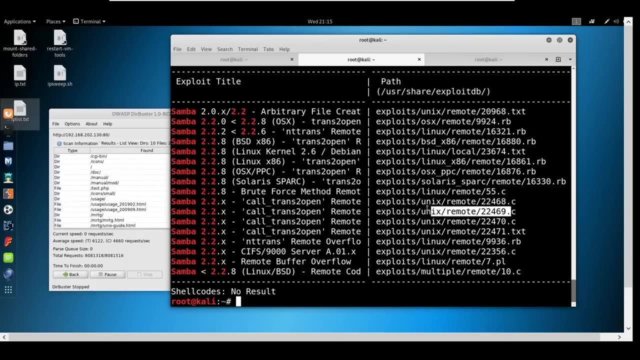 trans to open looks interesting. Again, this looks like an NT trans probably falls under that trans to open. There's a bunch of trans to opens here. These ones are all 2.2.8.. This 2.2.x trans to open again, And you can see that they're different types. So these are C files. We would 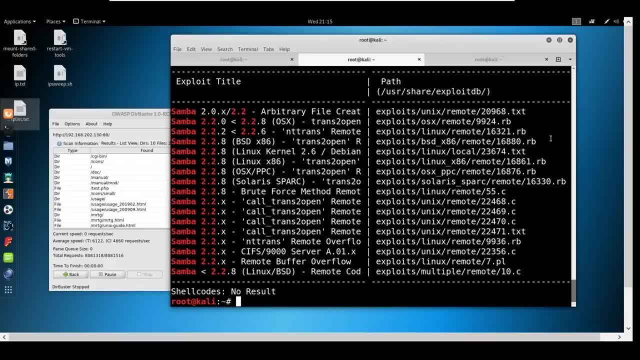 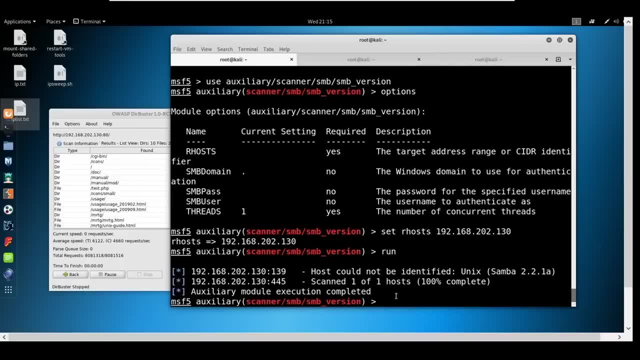 have to compile those ourselves. The Ruby files again, are likely going to be some sort of Metasploit module already existing, And if we came into here and we just searched trans to open, this is a quick way too if you're already in Metasploit. 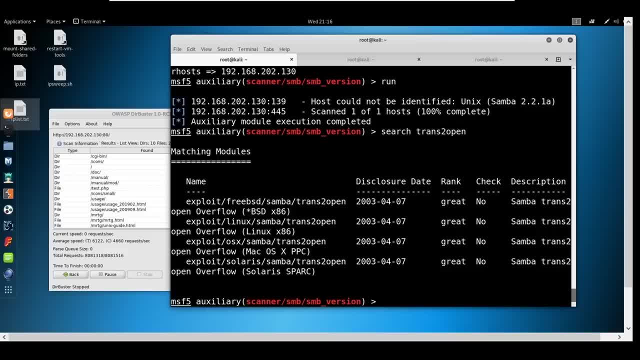 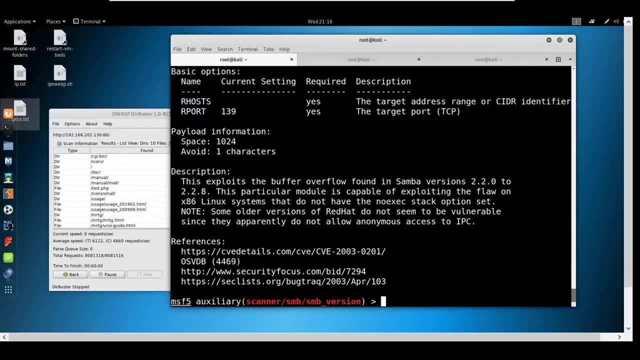 And we say, okay, search trans to open. You see that there is a BSD, a Linux, a Mac OS and a Solaris. We are on Linux. We could say info exploit Linux, Samba trans to open And get some information on this exploit itself. We don't even have to. 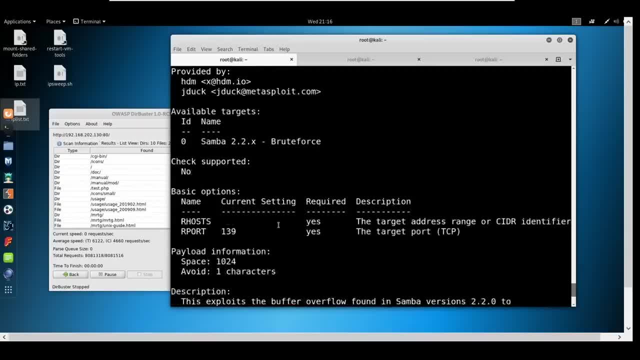 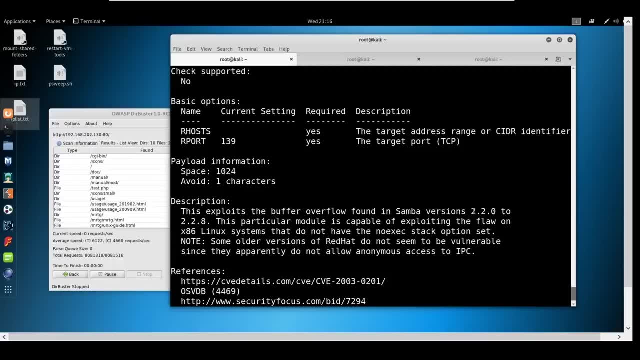 go out to the web to see this. So if we look at the description, this exploits the buffer overflow found in Samba versions 2.2.0 to 2.2.8.. This particular module is capable of exploiting the flaw in x86 Linux systems that do not have the noexec stack options set. Some older versions of 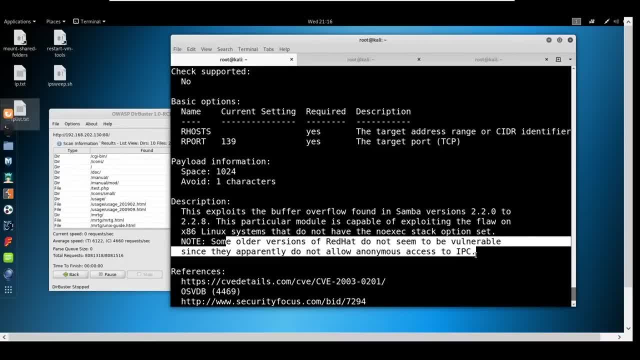 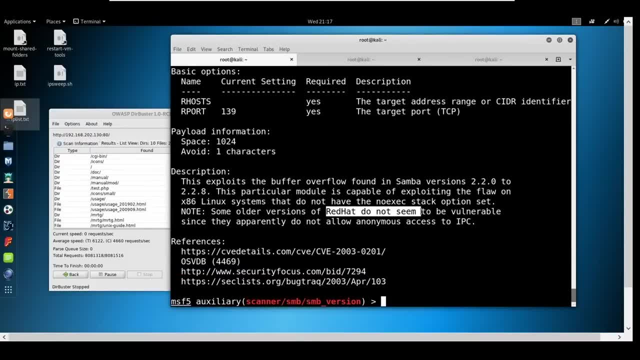 x86 Linux systems are vulnerable, since they apparently do not allow anonymous access to IPC. Okay, So we don't know specifically what version of Red Hat we're on, And we don't know specifically if this machine's running x86 or x64.. 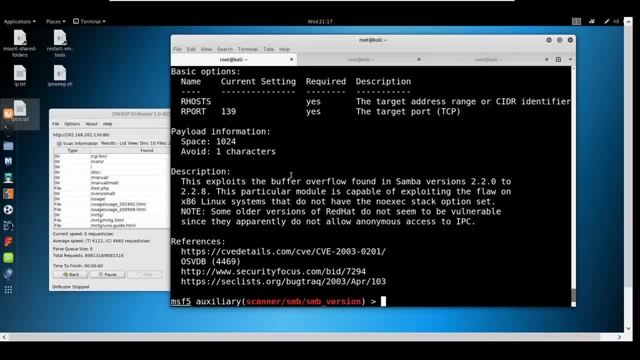 At this point. if this was a production system in a live environment, we would probably call up. if we're certain that this could be an exploit that we'd want to run, we would call up the IT manager or whoever is in charge of the project. 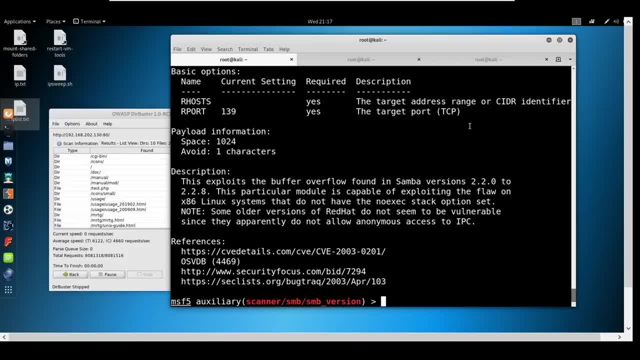 for the client and we'd say, look, I've got an exploit, I want to run it against the machine. Are you giving me permission to do it? As long as there's permission, You don't want to take out a critical server or something and then knock over a network. That's the last thing. 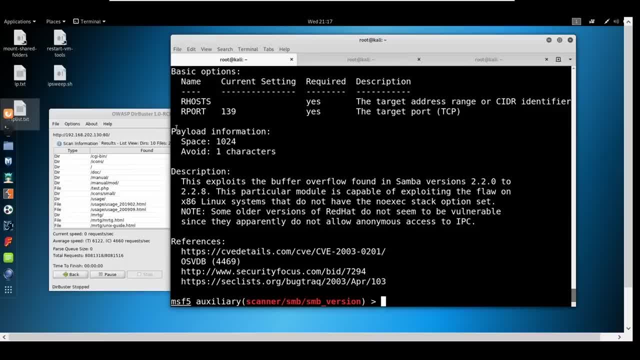 you want to do is deny service When it's typically out of scope. so, as long as you have the permission and they're aware that you're attacking, that would be the next step. So you would fire this guy off and maybe you would get a shell, maybe you wouldn't. um, and that's that's really it for. for this, i don't. 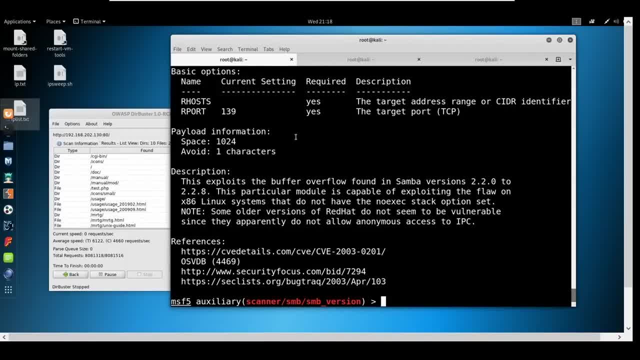 want to dive too much deeper. it's, it's just about. it's about looking at things and digging, and digging, and digging deeper. now, next week, what we're going to do is we're going to go into key objects again and we're going to start exploiting, and then we're going to start. 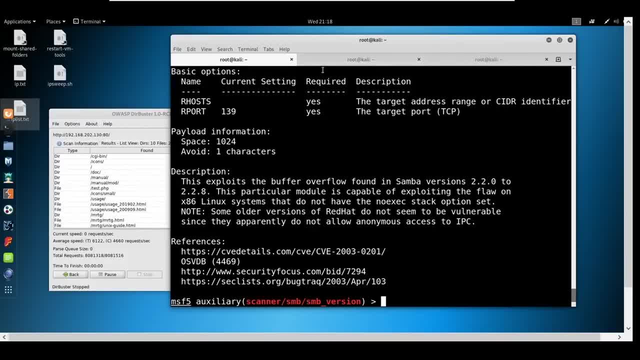 building our own exploits in terms of modification and compilation, or compiling exploits and really gathering how to get those on the web, and then, depending on how long i figure out that takes, we might actually dive into another module that i have planned, so it'll just depend on that. 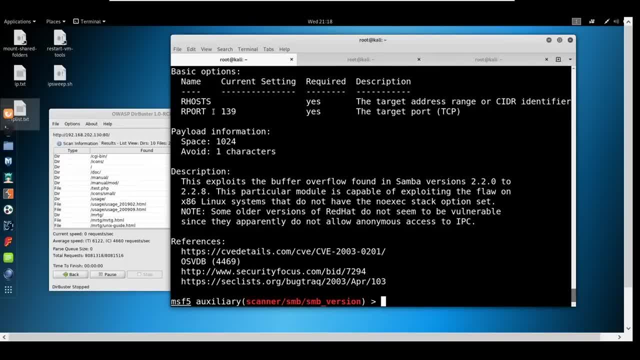 but from here i do want to pick a random box and i want to just do a scan on it and it may take some time. we may just do an ama while we're waiting. i'm going to pick a random box, we'll see what comes up for, hack the box and then we'll just kind of go from there. 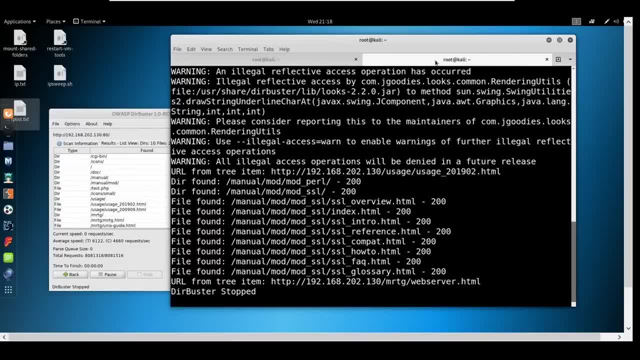 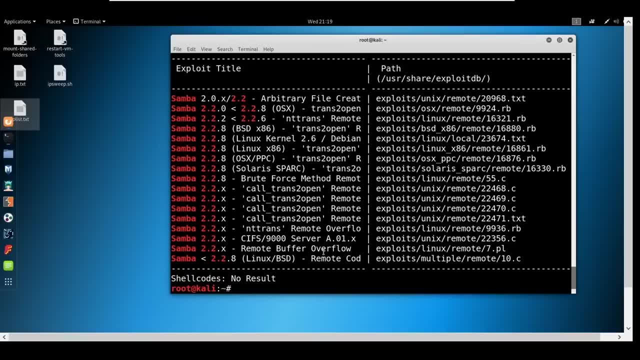 so i'm going to close out of this one, um, i'm going to close out of durabuster as well, and we'll we'll take this to to 10 o'clock on the scanning, and then we'll we'll drop and just go straight to ama. um, i don't want to beat a dead horse here. so if we are going to connect, 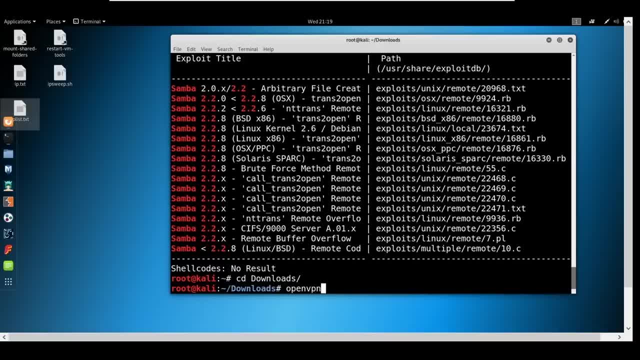 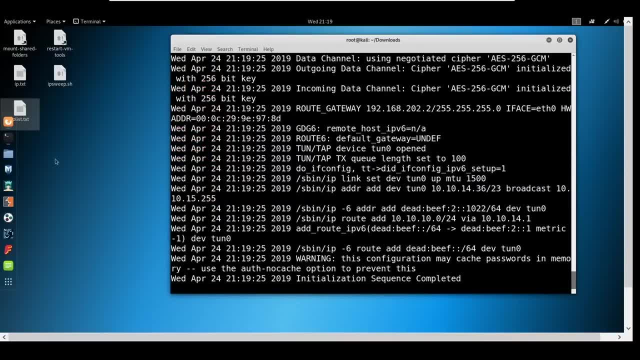 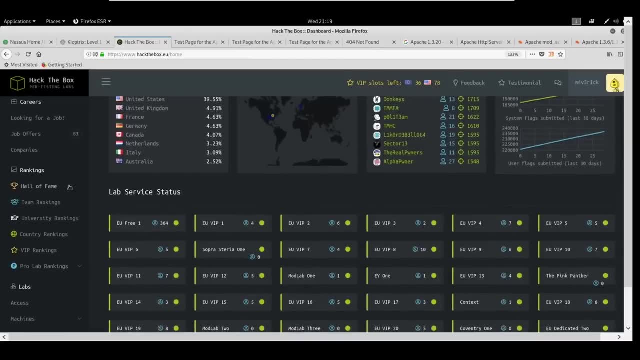 i need to get on the network, okay, and let's pick a machine. shall we any recommendations? and don't, uh, don't give me one just because it's ridiculously hard. i'd rather have one that has some decent output. active, active is is not, uh, active anymore. 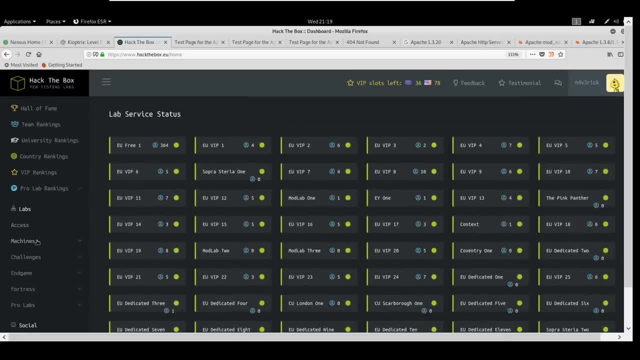 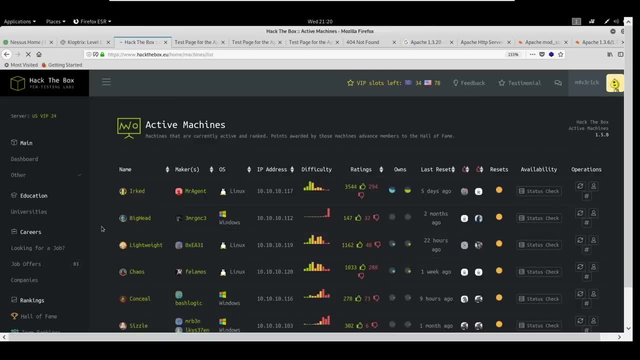 unless you just mean an active machine. we are not doing retired, we're. we're going to do active machines for the sole purpose that we're only enumerating. i'm not going to give any inclination. if i think something is an exploit, i'm not going to give any explanation at all. i'm going to say this looks interesting. 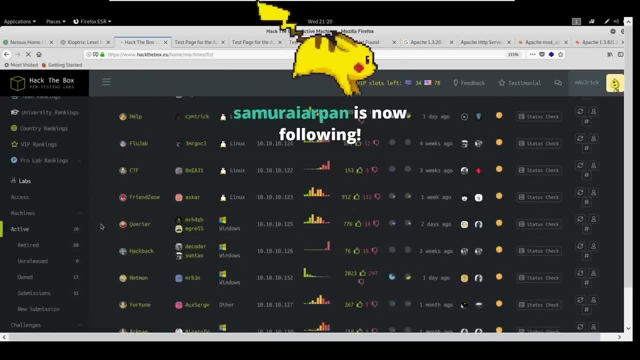 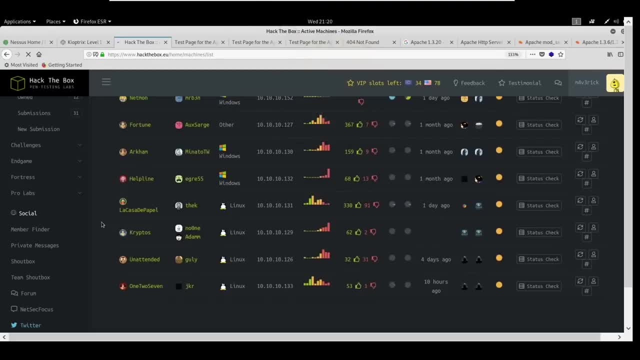 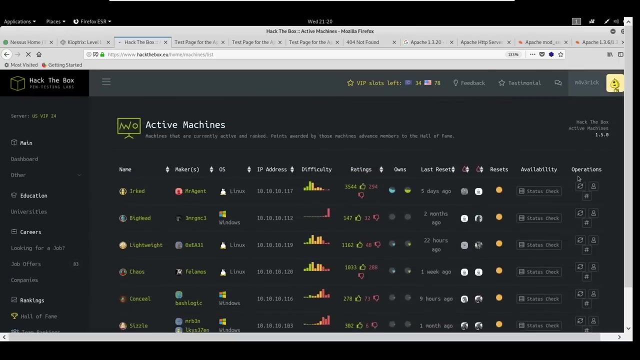 this doesn't look interesting. um, that way, you guys don't cheat the system. one two seven. everybody's saying one, two, seven. all right, we'll do one two, seven. as you can see, i've never done this. i think i'm actually. am i machined out? i am machined out completely. look at that. i'm terrible at hack the box. 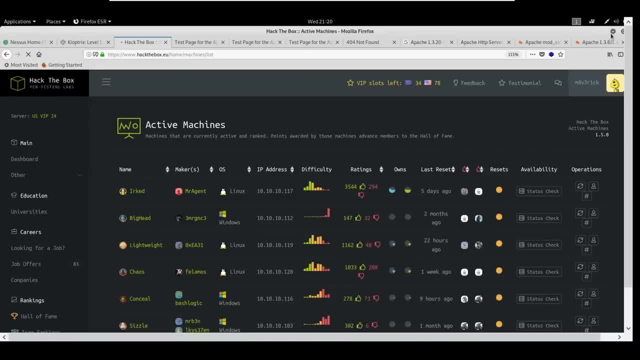 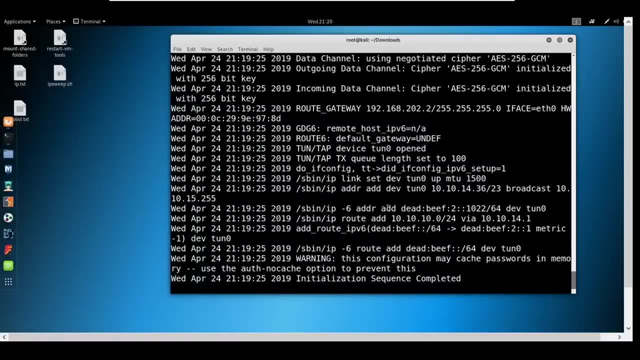 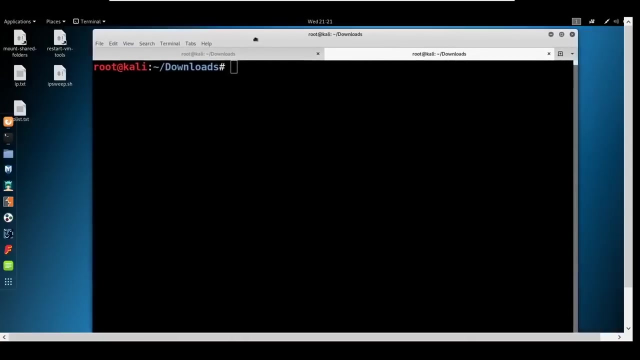 okay, we'll do this guy. if it's truly against the terms of service, then i'll. i'll take the fall for it. i'm not concerned terribly. if they ban me, then they're. they ban me and i lose. i gain 13 a month back, i guess. 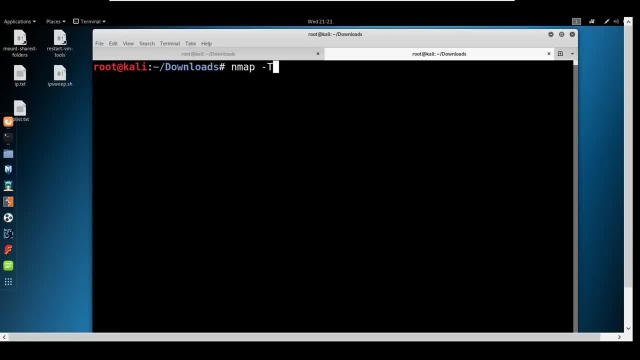 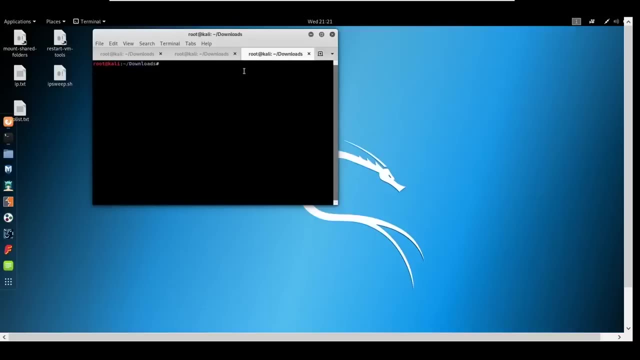 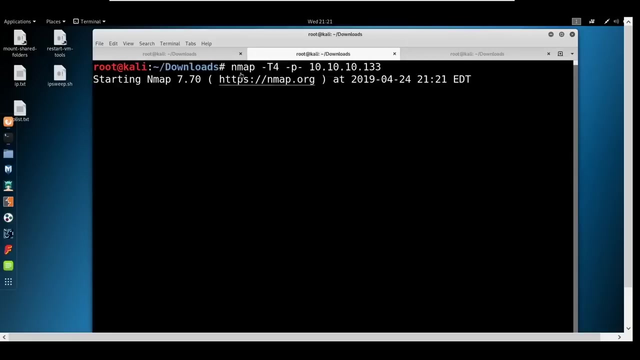 all right, so we're gonna do our scan t4 all ports. also, one thing we didn't do that we should do. i just didn't do it because i i'm aware of what kiaftrix has to offer. um, when we're doing these sorts of scans, we should also be scanning on. 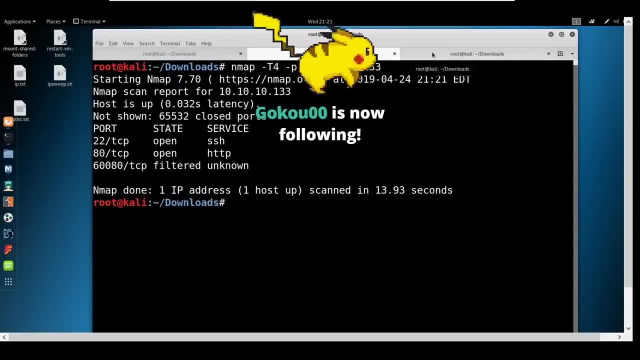 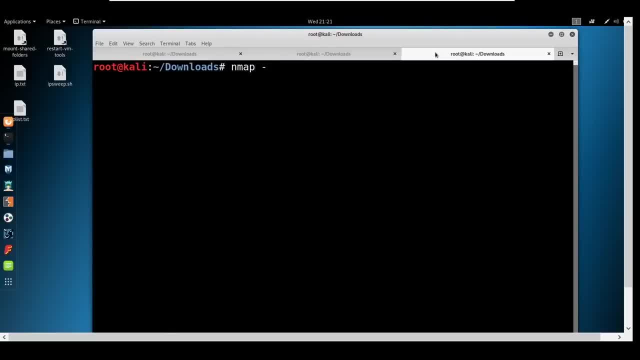 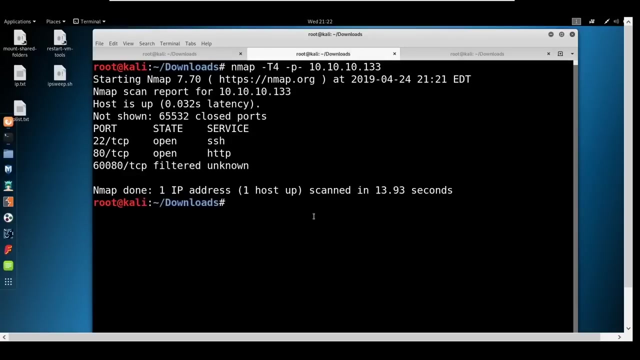 um on udp as well. so we're gonna do su t4 all, no, not all- ports. we'll leave it top a thousand. all ports will take forever. don't ask me what i was thinking there for a second. i'll run that, okay. so the quick scan came up with with three. we're gonna change that now to 2280 and it looks. 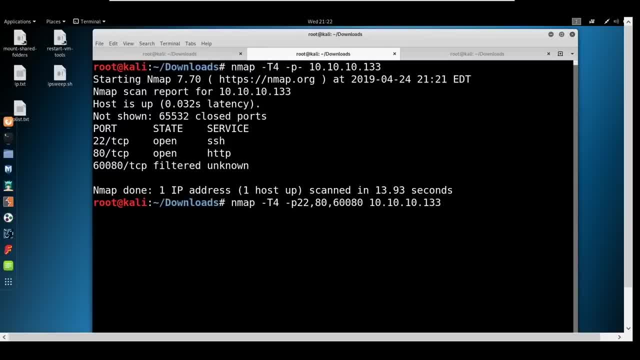 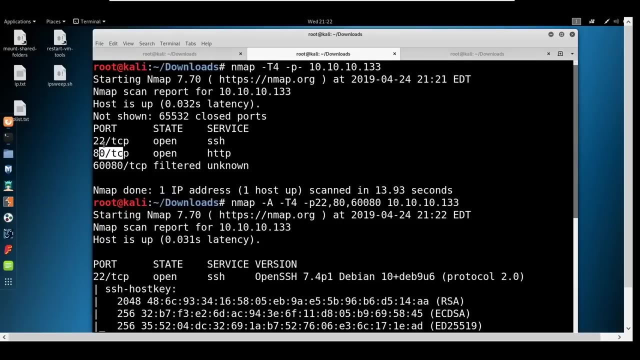 like a filtered port of 60,080. uh, we're going to change that to a dash a, so we'll see what that is. okay, so my my experience doing hack the box, doing capture the flag events and many, many oscps. i don't know if this is correct, but when i see 80 and i see 22, my immediate guess is that you. 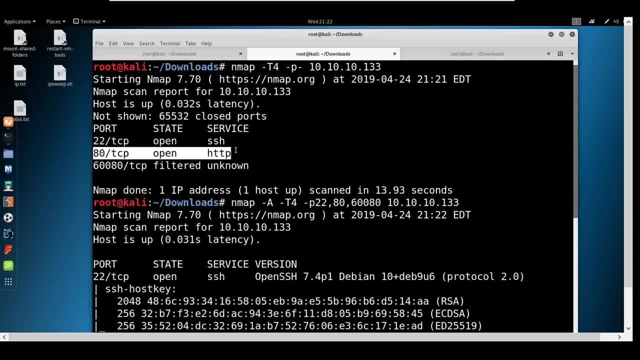 find an exploit on 80- that's going to be the one. that's going to be the one that's going to be- that leads to some sort of credentials. those credentials will lead you to port 22, which allows you to log in and get a shell. that is not always the case. sometimes we'll have an exploit on. 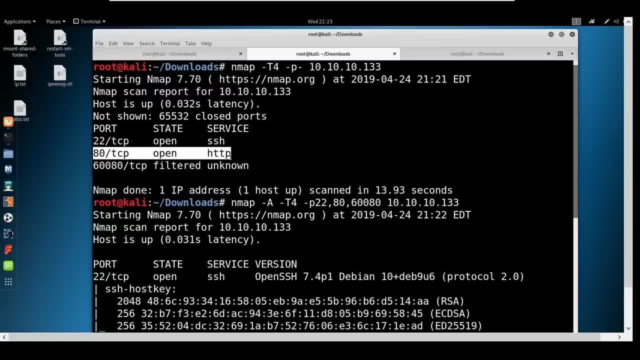 80. that actually gets us remote code execution. we'll find credentials and then we'll ssh over and, uh, get root. um, there's quite a few paths. this six 60,000 port up here is also interesting. um, so i mean just just looking at this from a capture, the flag event point, i'm not sure if it's. 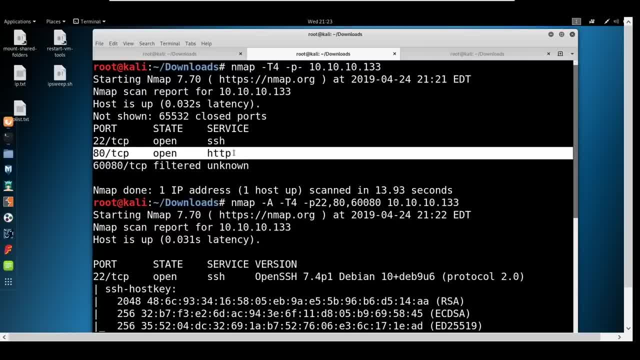 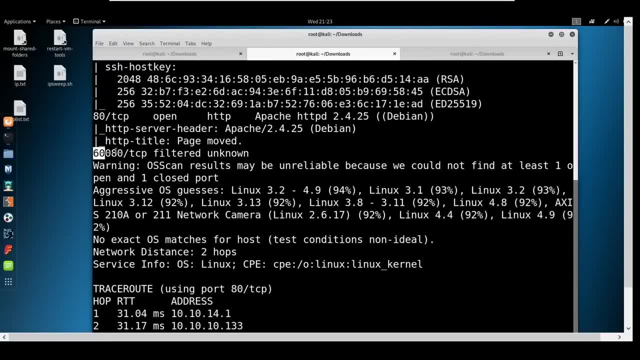 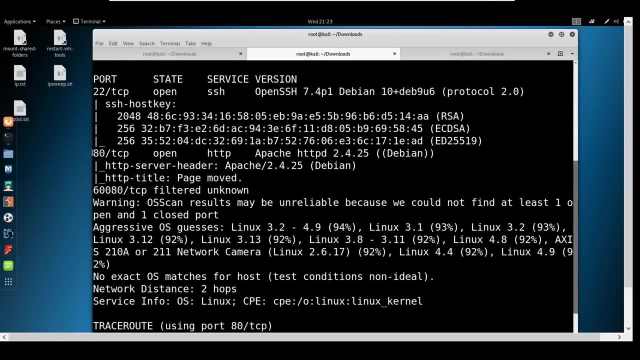 a flag standpoint. my first and big focus is this: port 80, especially as this is filtered, um. so again it's coming up, filtered, unknown, we could try to, to netcat or telnet, to this, which we haven't talked about. netcat yet, that's next week, um, and so it looks like port 80 here. 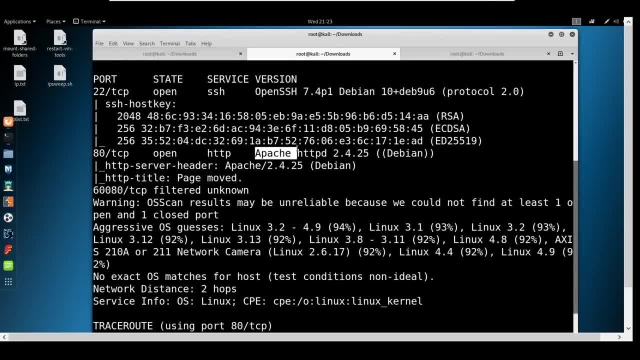 and if we're doing this from a pentester point of view, again, we're getting server information httpd coming through the server header. it says the page is moved. okay, so we got a little information. what we see. um, this would be a finding right? we talked about that already. 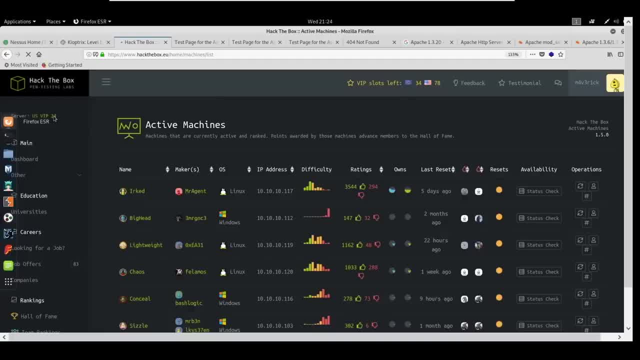 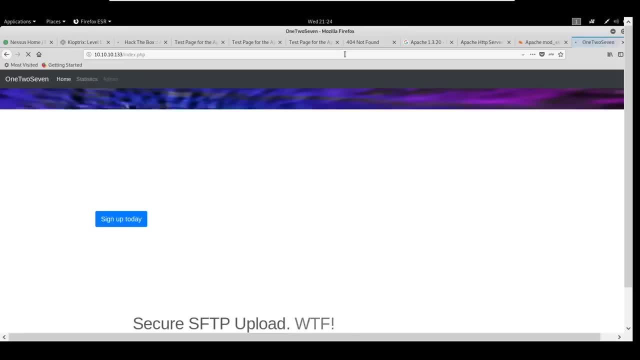 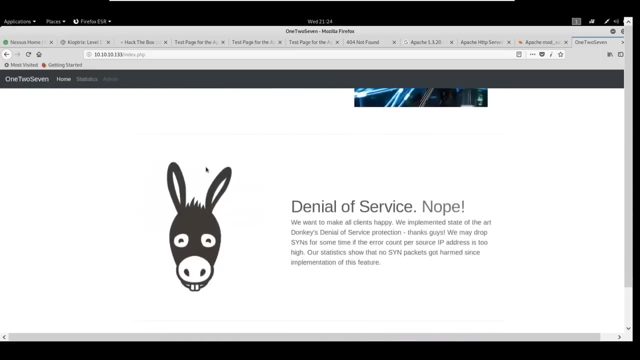 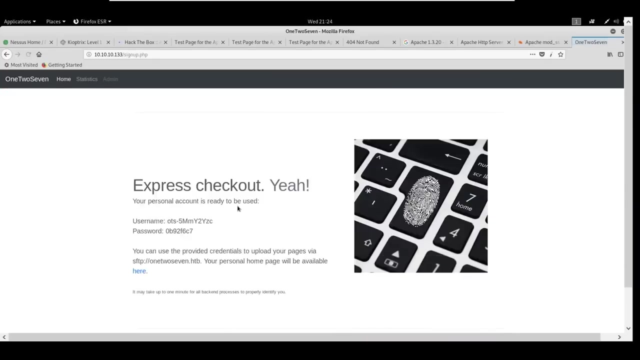 information disclosure. so let's just go ahead and go out to the the website and see what's out there. okay, it looks like we redirect as soon as we get to the page. now we've got, uh, we got a page here. looks like there's a sign up page. it gives you a username and a password. 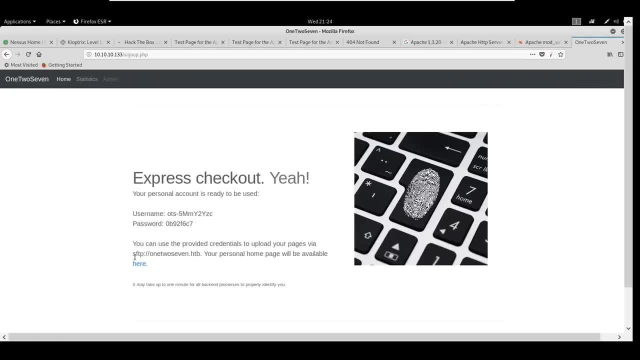 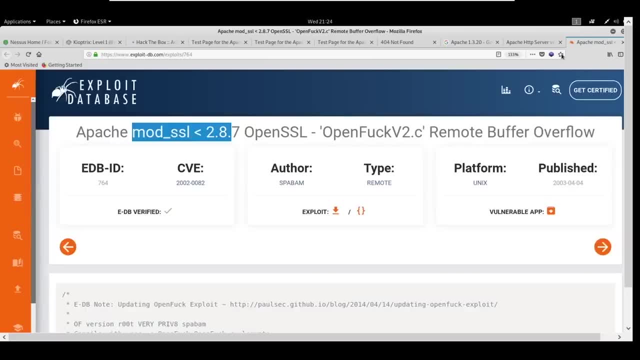 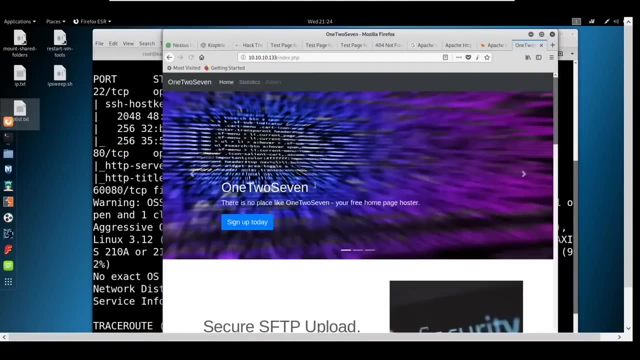 credentials to do sftp. your personal home page will be here. we'll just click around. looks like we may need to add, and i just closed out of it. we may need to add something in our etsy host to resolve that, or we make it work ourselves. 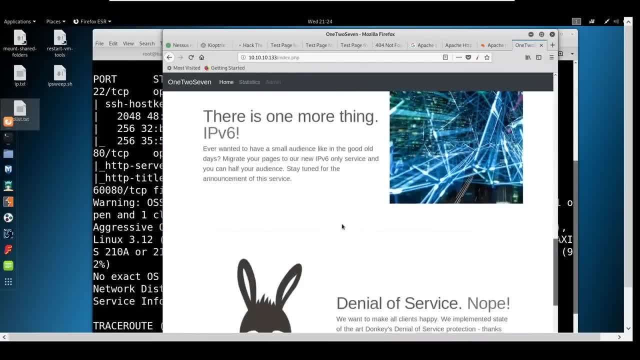 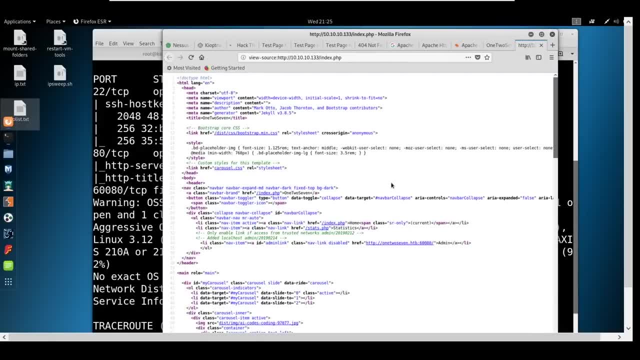 um, anyway, let's not get too ahead again. i don't want to get into exploits, so a couple things that we're going to look at. we'll view the page source. uh, looks like they're running jekyll, which is like a common um common blog post type. uh. 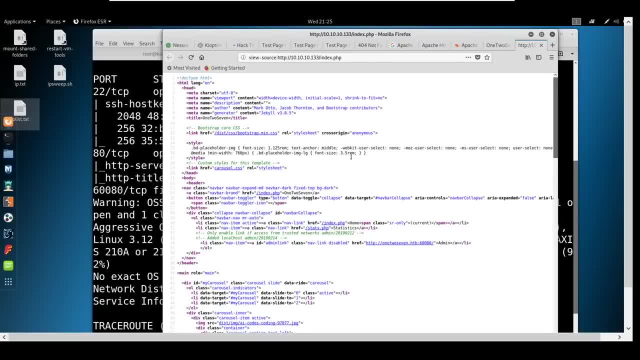 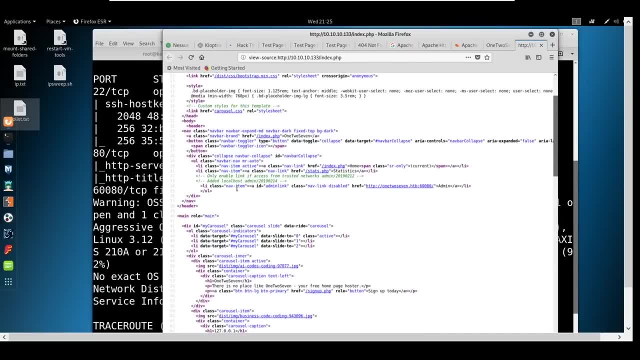 framework, i guess, is typically where i see it. ah, look the admin link so that that 6080 right here, that port 6080 that just showed up, is showing up here and this is um showing 127.htb. and when we have something like this, we need to. 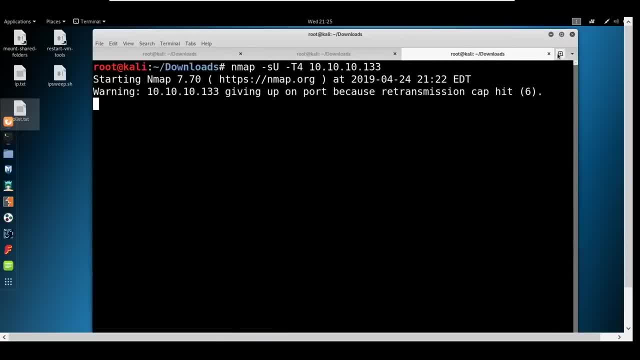 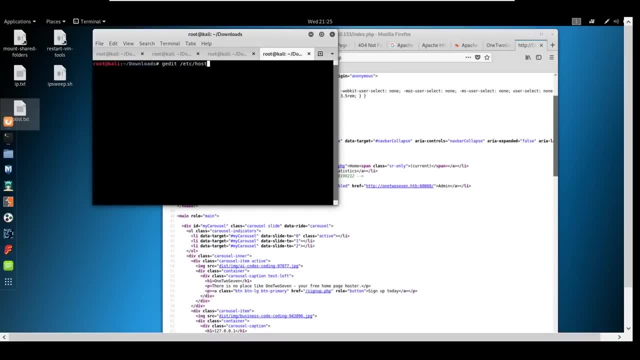 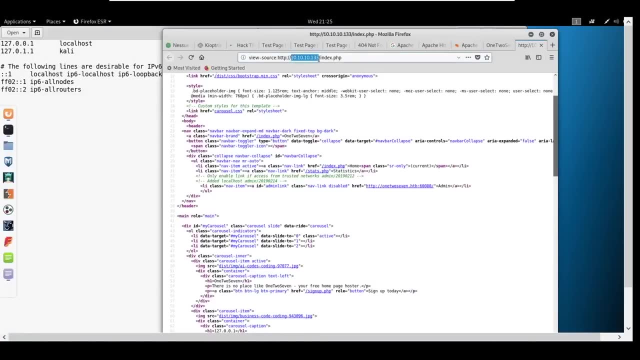 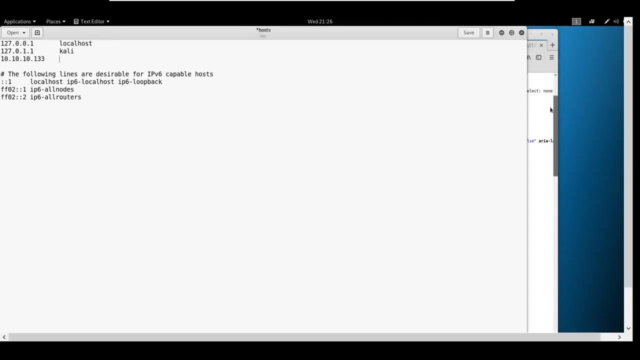 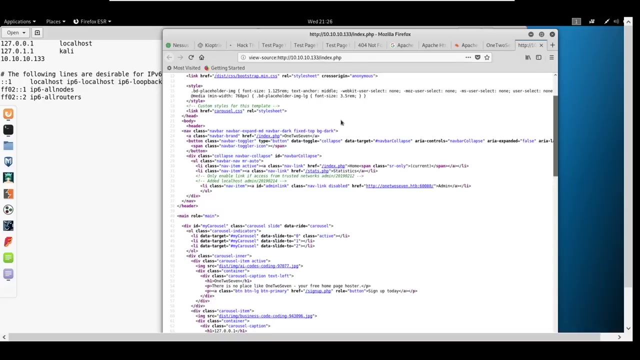 okay, we just need to modify our etsy host, so so, so, so, so, so so. and for those of you who are not aware what i'm doing, i'm changing my dns local dns record here, um, so that way we can access this page when it goes 127.htb. 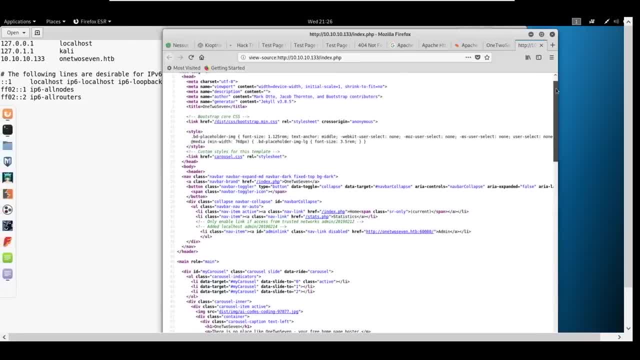 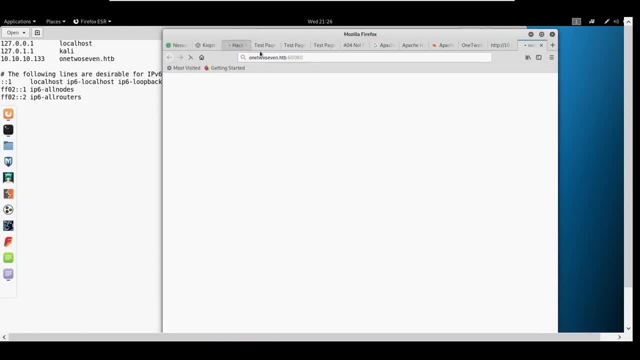 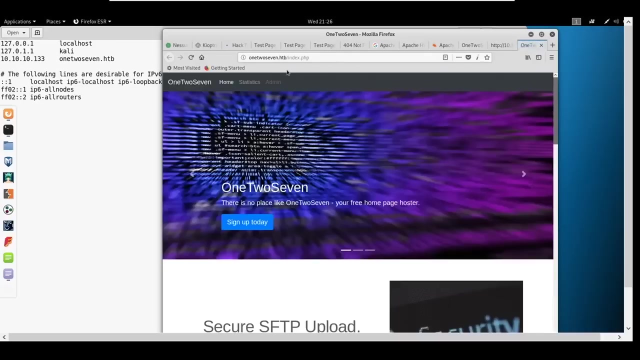 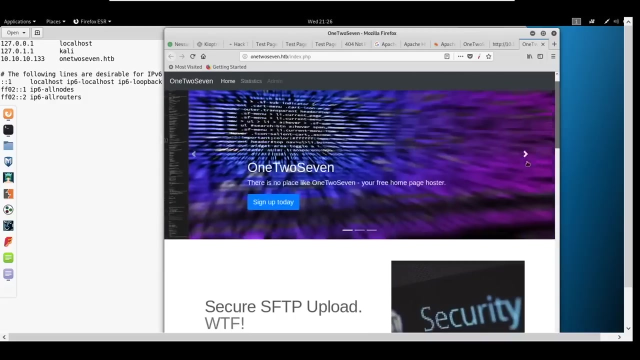 okay, let's see if we can get to this page in a new tab. delete that, and it may not work because that port is filtered. let's see what happens. okay, so 127.htb is now working. um, so, that's good. so there's some, some pages here we typically want to click through. 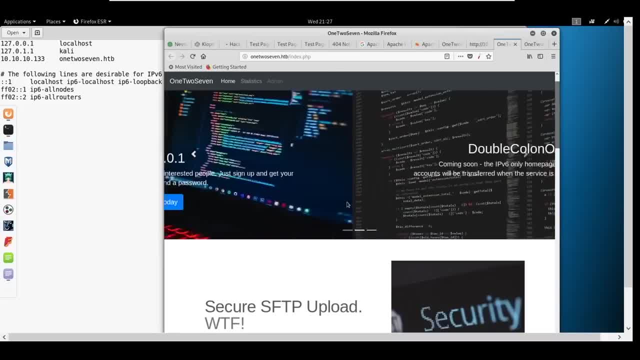 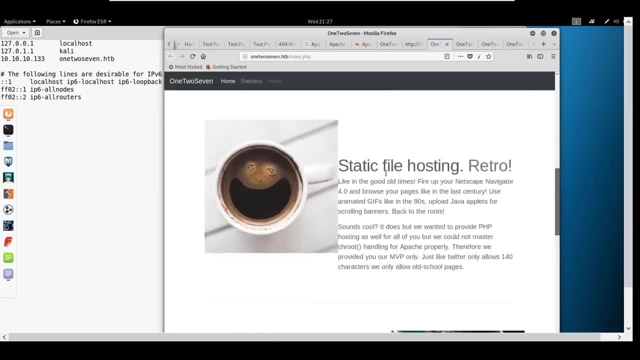 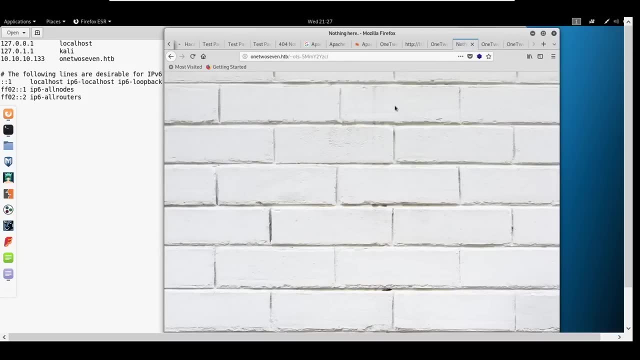 uh, sign up today. sign up today. i'll open all these and just see what's going on. secure sftp upload. sounds like there might be a file upload here. let's click on this and see what this is. so it took us to a page, okay, so 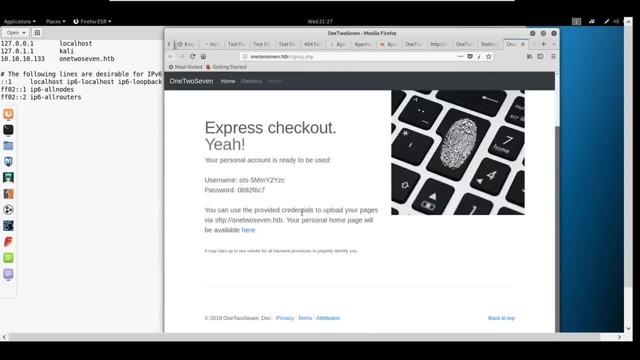 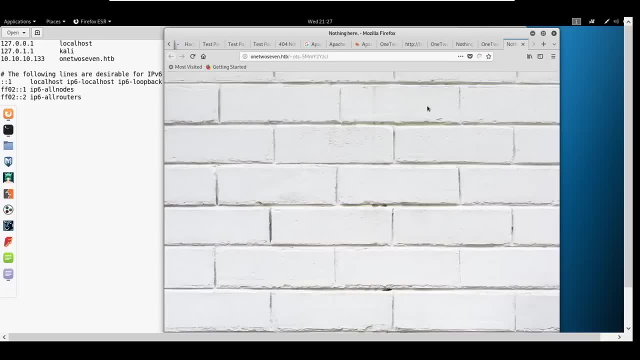 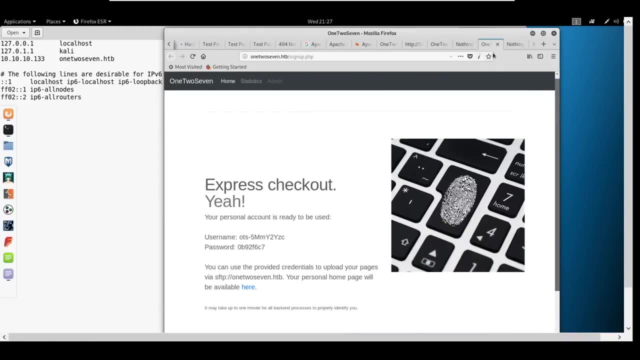 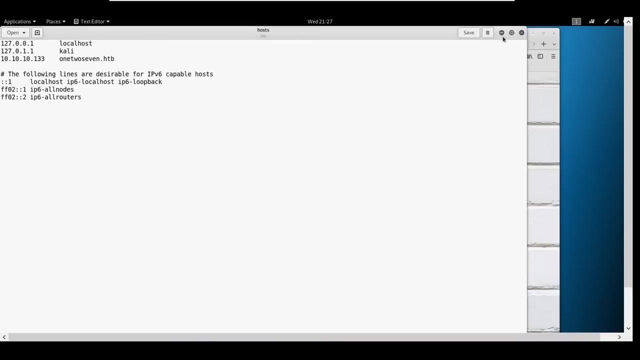 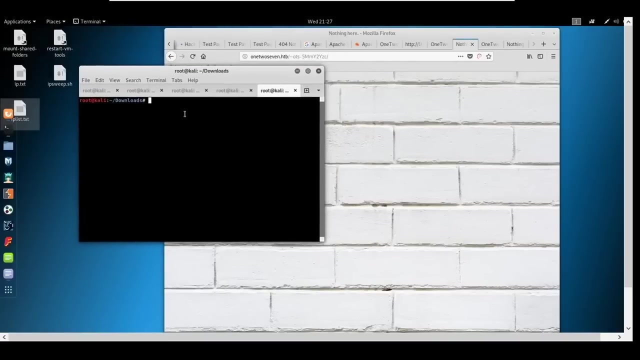 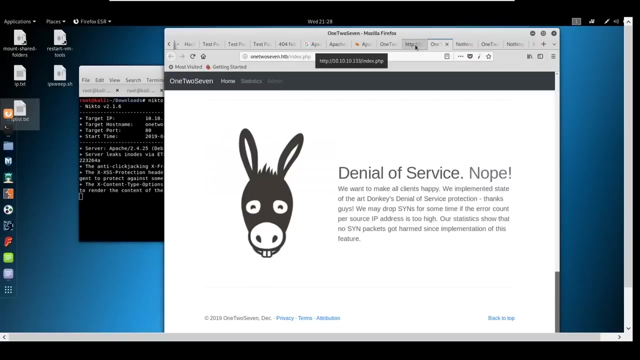 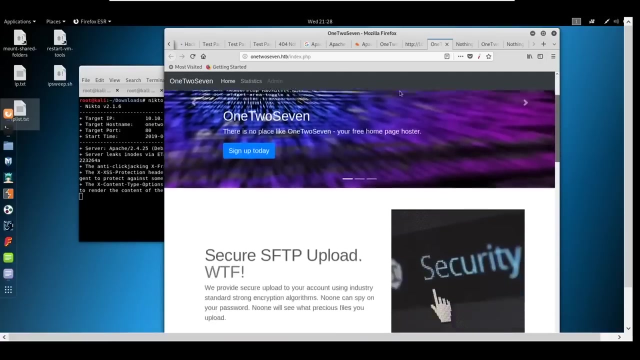 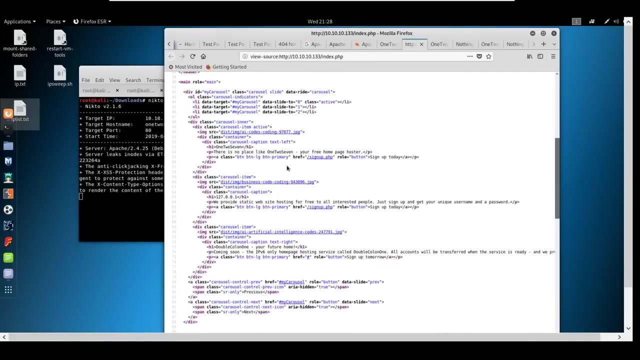 so, so, so, so. so let's, let's hold the standard here and let's do a nycto real quick on the host. we can also run a durabuster if we need to. i'm just going to read through the source code real quick while that's running through. 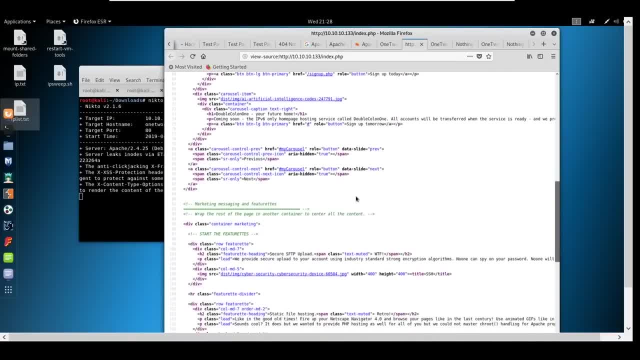 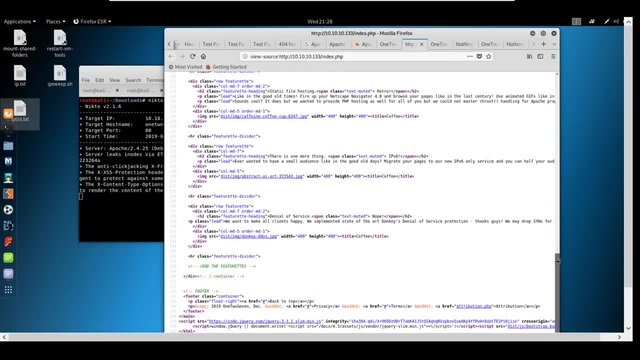 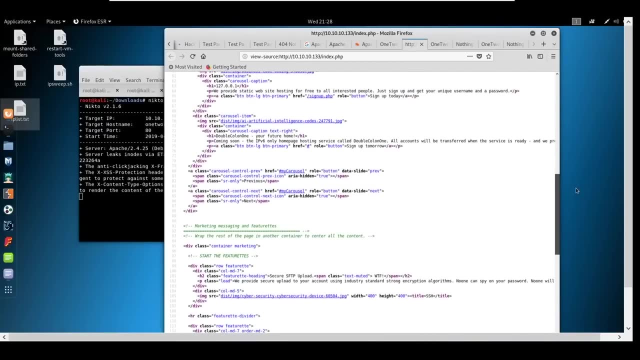 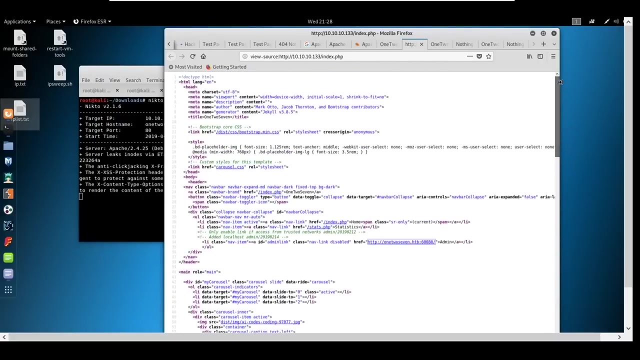 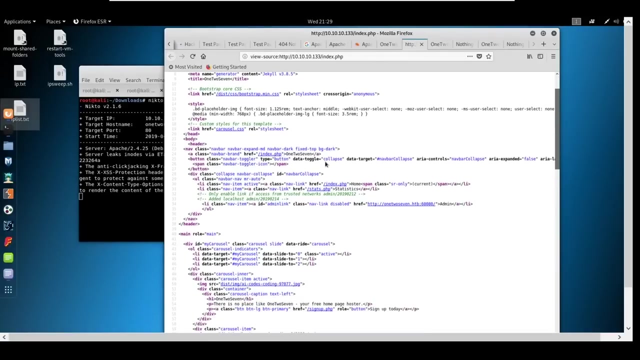 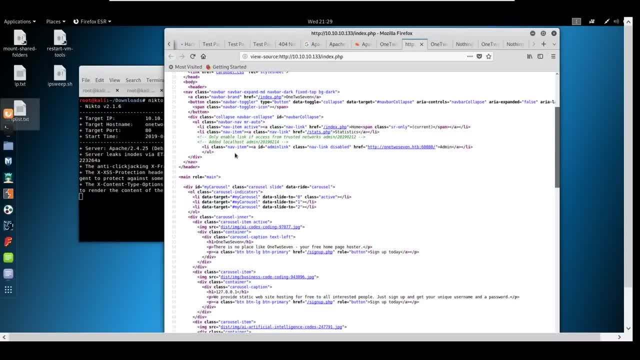 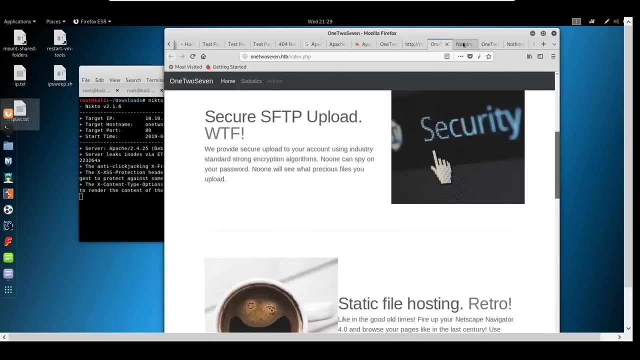 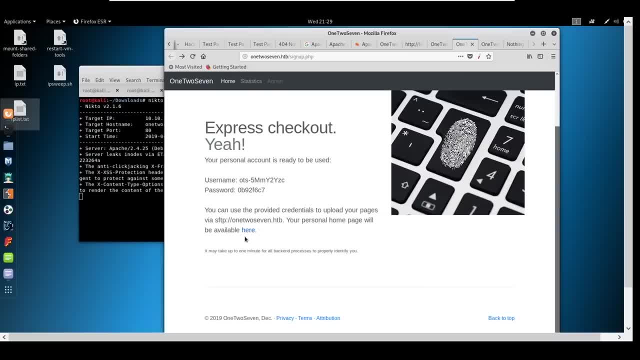 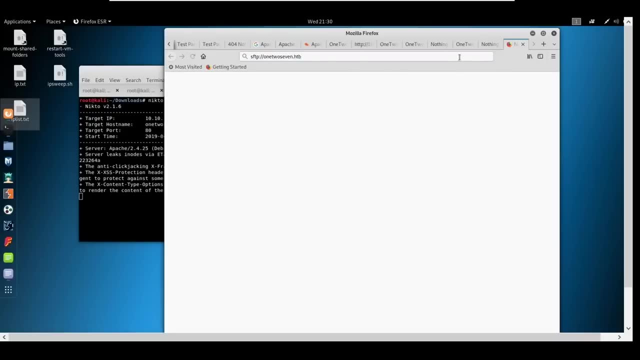 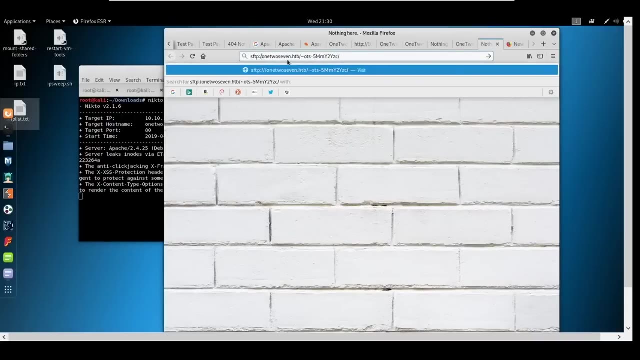 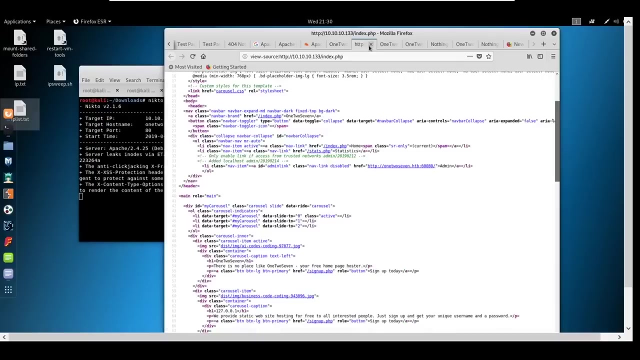 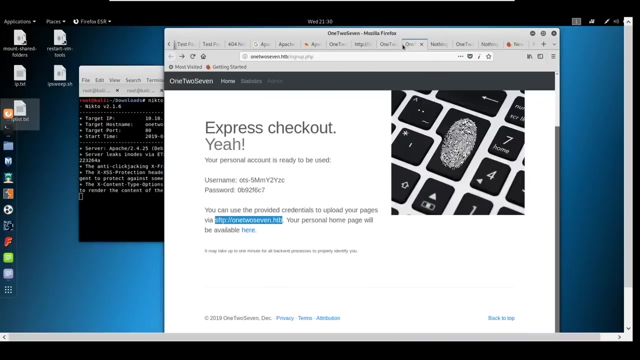 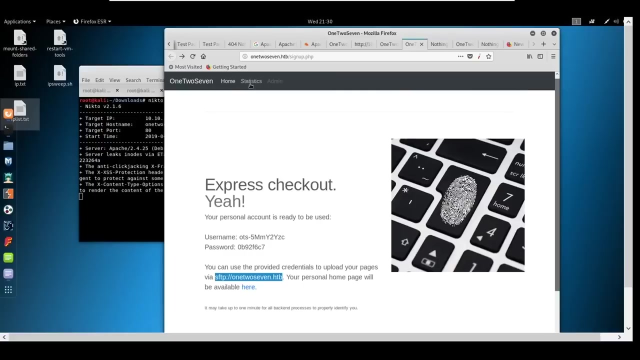 so, so, so, so, so, so that's not working either. um, so it looks to me. i don't think it's stego i. i think somebody says cli, i think it is cli. um, so it looks to me, and i don't want to give away, so i'm not going to tell you what i what. 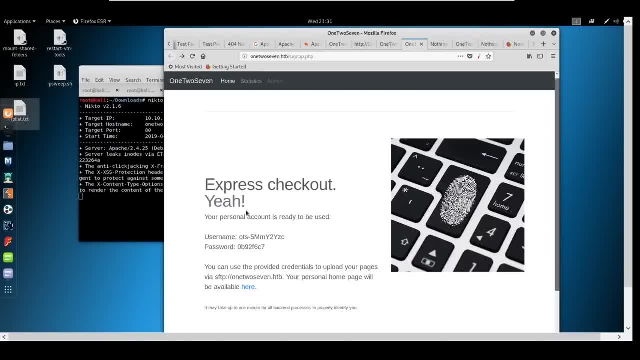 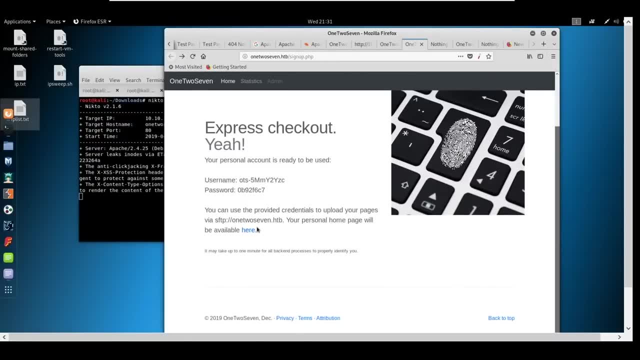 i think is going to happen here, um, but there is a file upload. if i had to guess, there's a vulnerability in the file upload that allows you some sort of code execution that gets you into um, at least into a lower shell. you're going to have to somehow get into the. 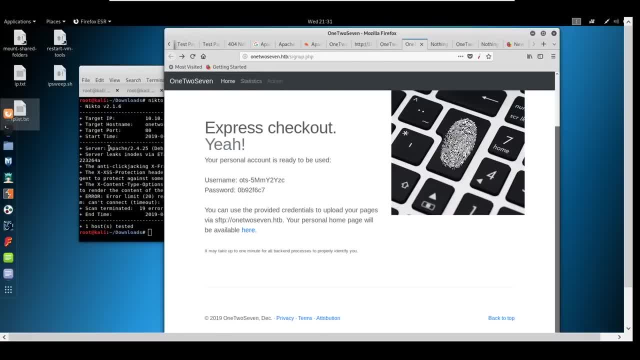 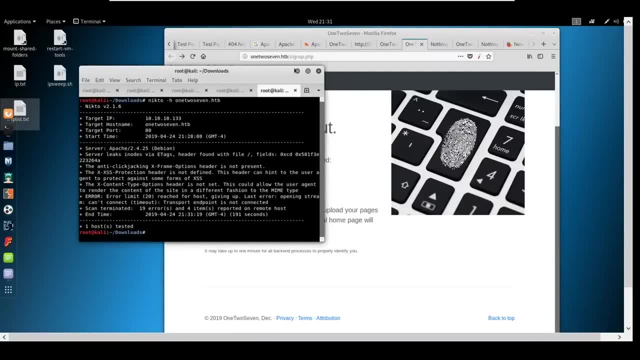 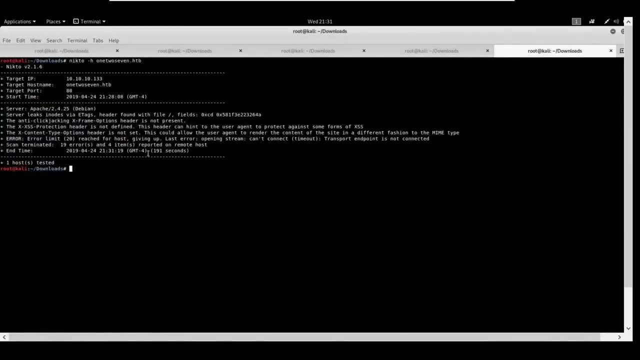 admin page at some point in order to get that, uh, that full access would be my guess. um, so when we're looking at this too, all right, let's, let's blow this one up, okay, so we found the server again. etags again, remember, those are pretty much low. 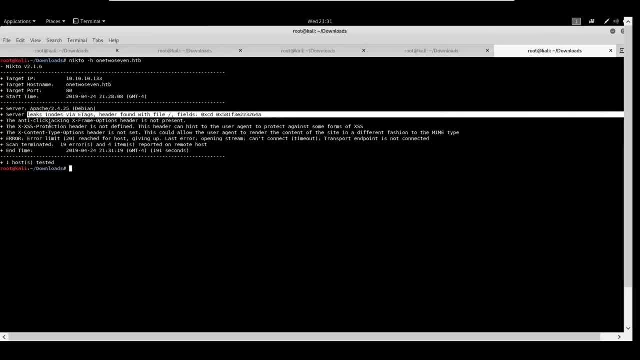 findings. i wouldn't put this on a a external report. i'd maybe put on a web app if i'm desperate. um. same thing goes for these headers again, and it looks like we aired out um on the rest of it, so we didn't get a whole. 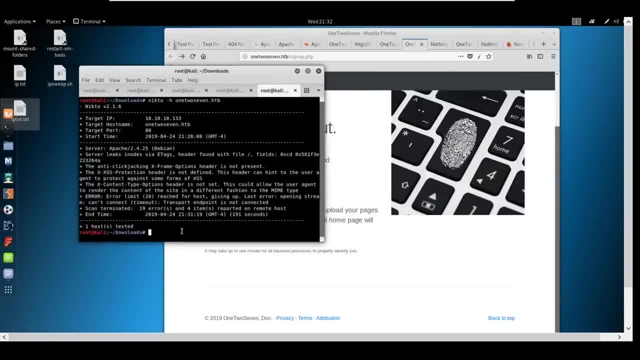 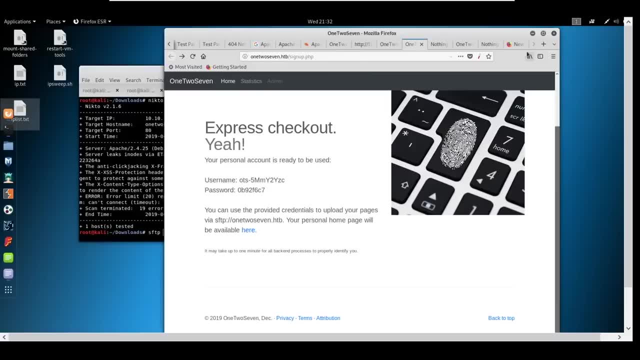 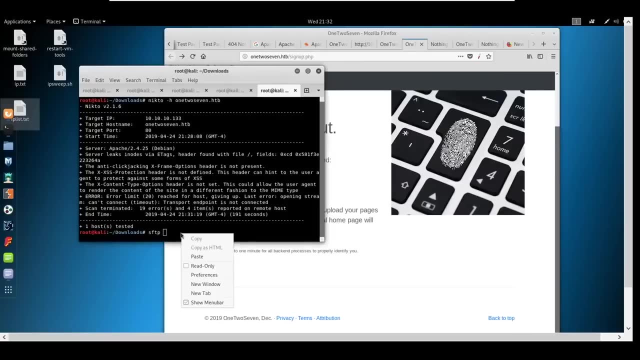 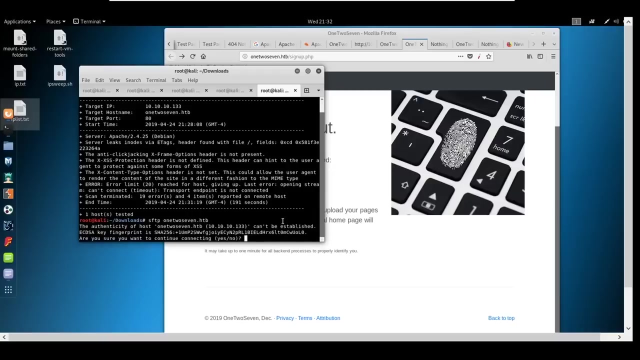 bunch of information. everybody's saying we should sftp through the terminal. let's do that as well there. so i'm going to do that. you guys can also hang this up right here and then just show me the only one that we've got. i'm just a little worried about. 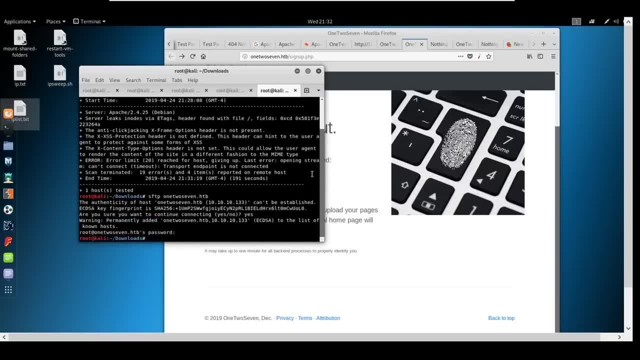 something like that, but it's something a little different, so i'm going to show you how to do this. we're going to open this up, ok, and we're going to read the header and we're going to see that this is going to be the end of it. 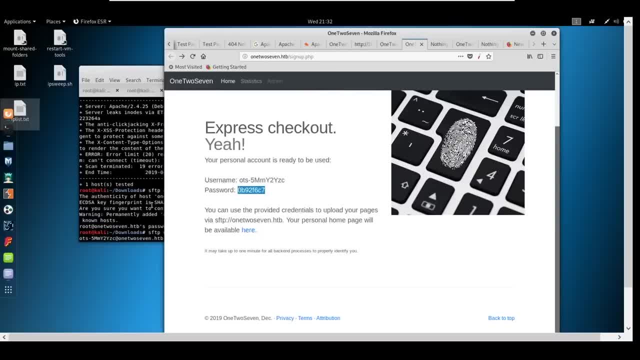 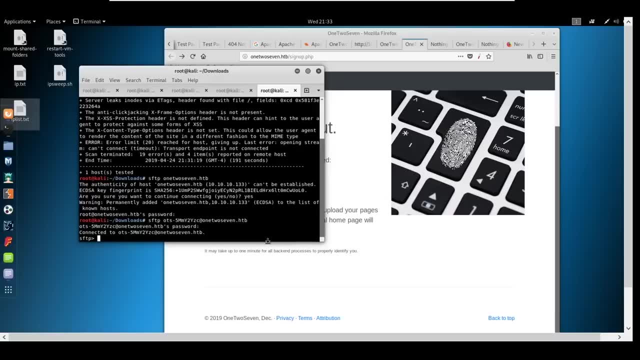 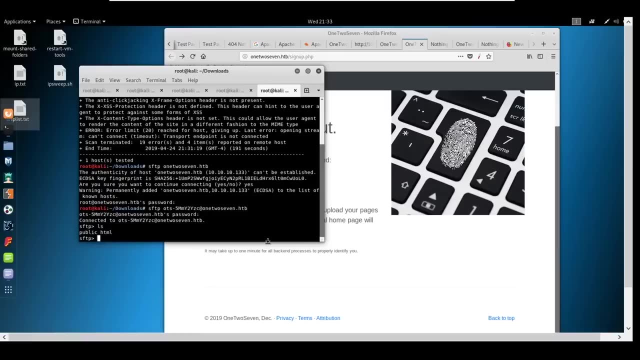 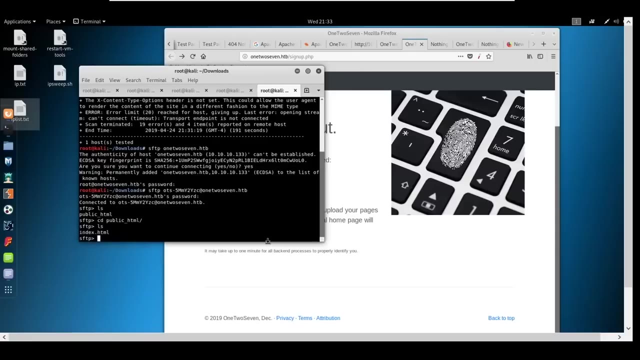 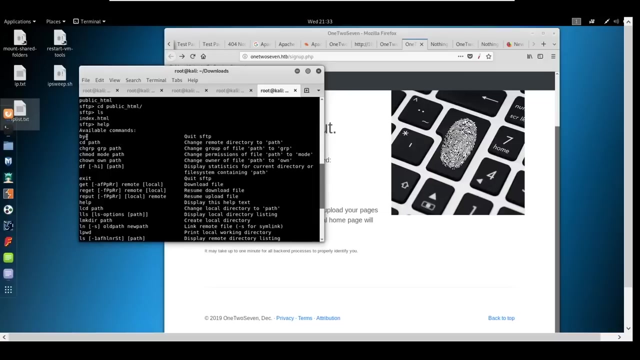 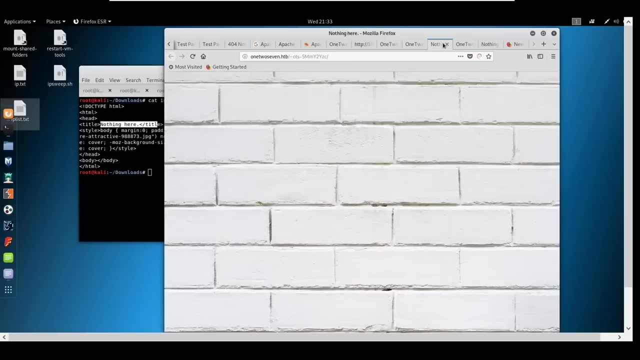 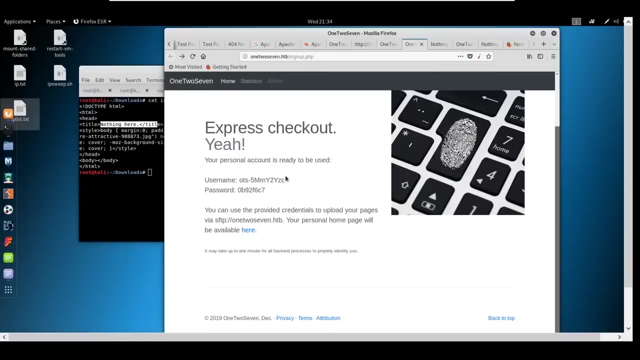 All right, we're in, Let's see what options we have. Nothing here. Ah, this is our web page. Does that make sense? So what just happened here? So they gave us our own personal web page And they gave us an account to log in via SFTP so that we can upload. 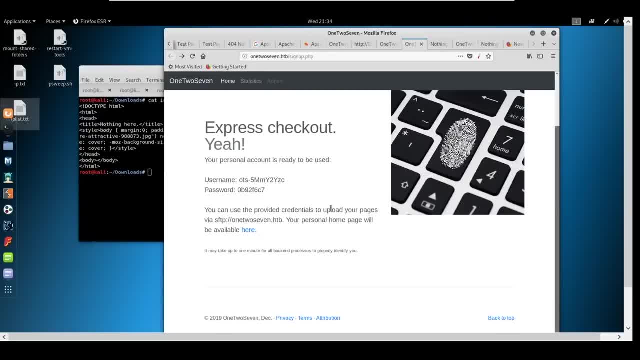 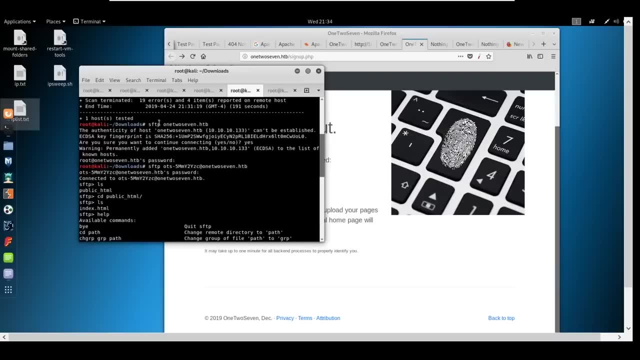 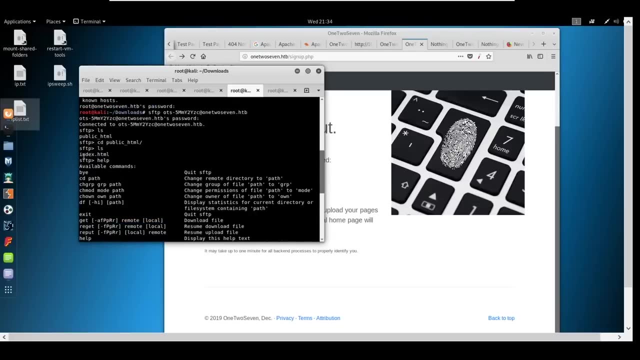 Focus on the upload. So we are in SFTP, which is in a public HTML folder. We have control of what we can upload into this folder. You see this indexhtml And when we catted it over here, it said nothing here. 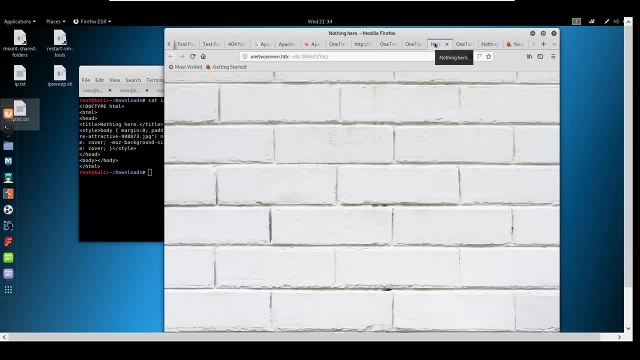 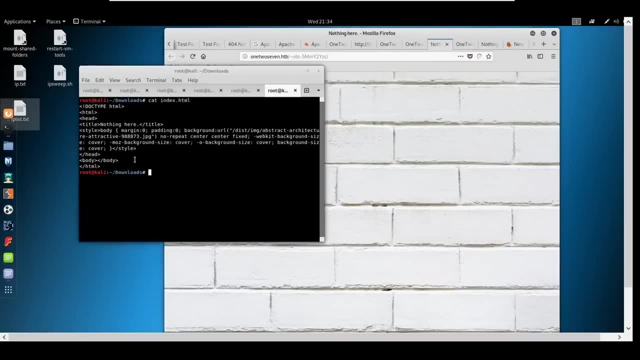 Well, what also says nothing here? Our home web page. So we're in SFTP, So we're in SFTP. So if we were to modify this home web page, we could probably put whatever we want. They've got the bricks in here. 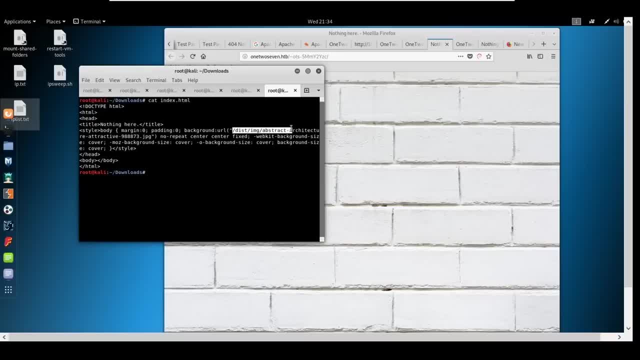 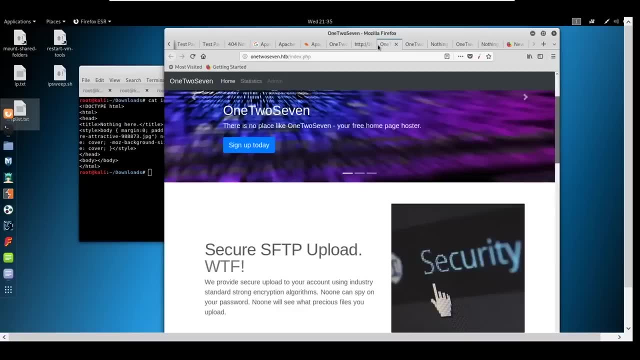 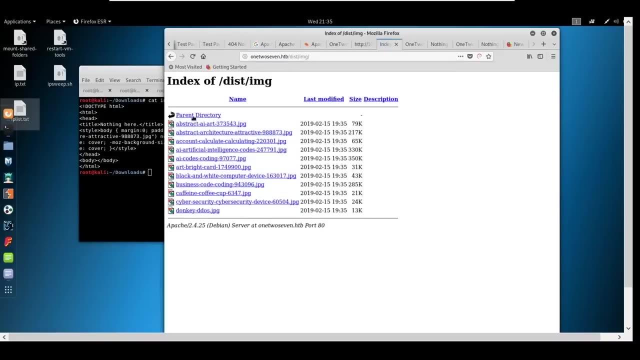 And we got a little bit of information disclosure as well. You see, they've got the abstract architecture JPEG. We could try to navigate to this folder area as well. Who knows if it's going to let us. Okay, so it does give us a parent listing here. 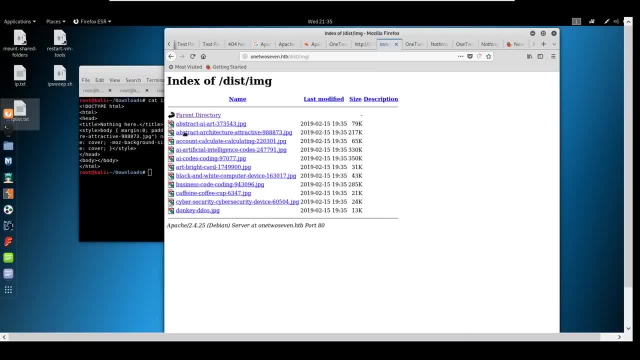 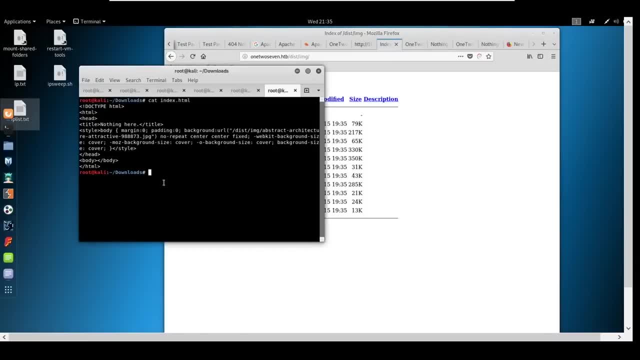 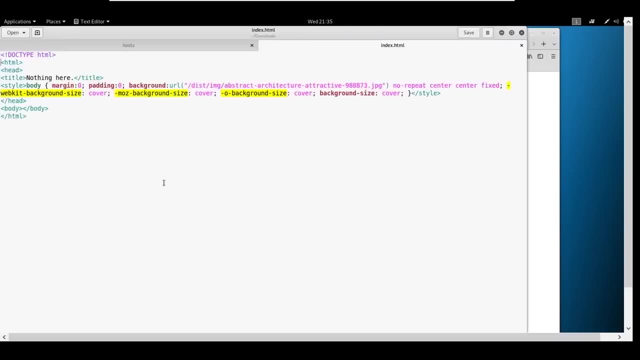 JavaScript CSS. So there's a donkey DDoS here. So just for proof of concept, yeah, let's just gedit this file, Let's change it to the donkey DDoS. I don't even want to look at it. 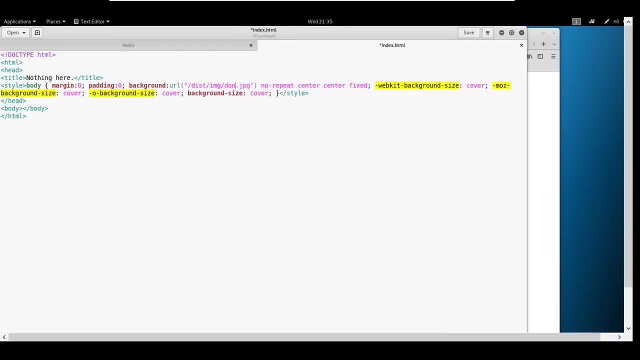 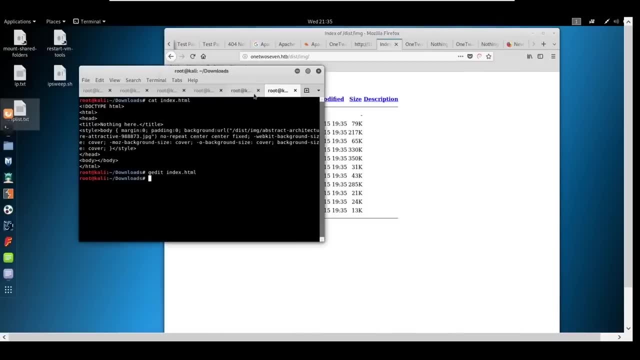 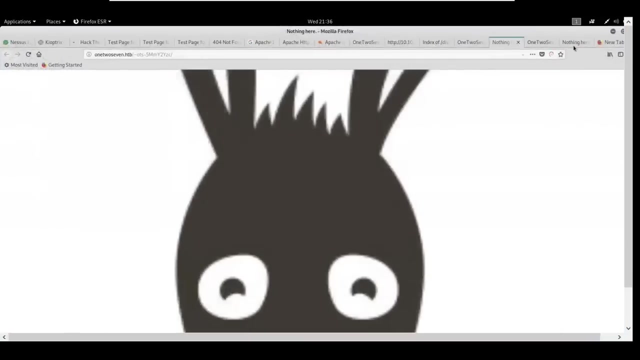 I just want to see what it comes up as: All right, Do we have a put, We do have a put. All right, Here goes nothing, guys, Here goes nothing. Hell yeah, We got a donkey now, All right. 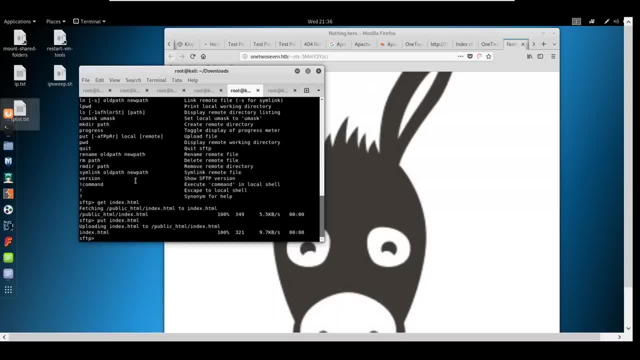 So we are proving here that we have full control. We have control of an upload of a source, We have control of a server that's Apache. That's as far as I can go, without saying where I think it goes. I don't want to get into exploitation. 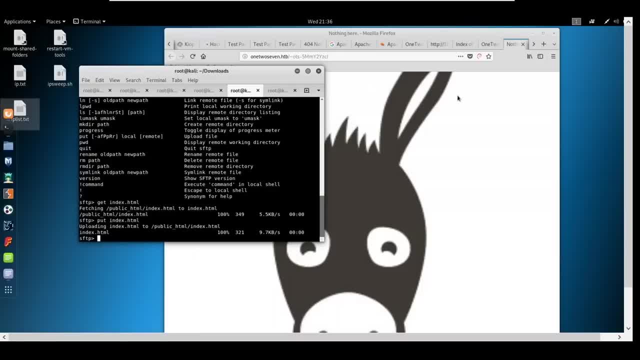 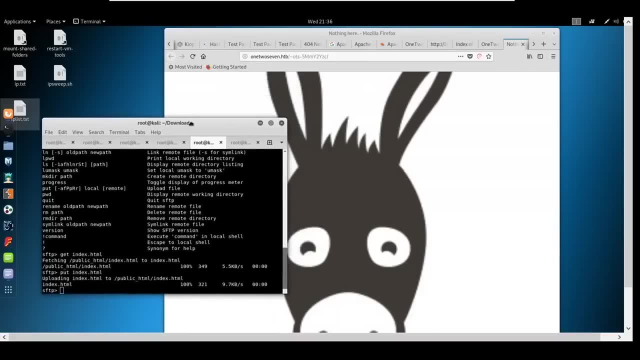 But I think the logical step. I've got a good feeling where the next logical step is. So if you are familiar with exploitation, your wheels should be spinning here. You should be thinking of where the next logical step is as well, But for the purpose of not violating terms of service, 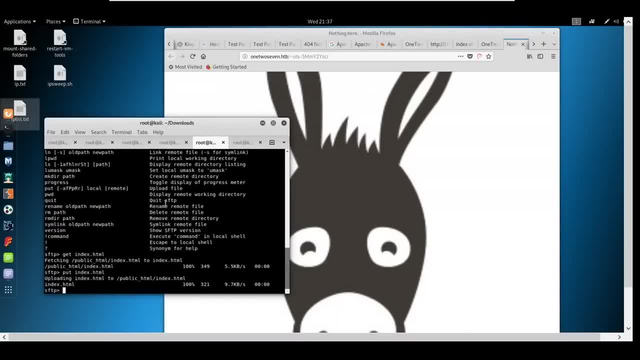 I'm not going to go any farther because it's going to require an exploitation attempt to be able to see if I'm correct in my thoughts. And if I am correct, I don't want to dig deeper. So that is an example of enumerating as well. 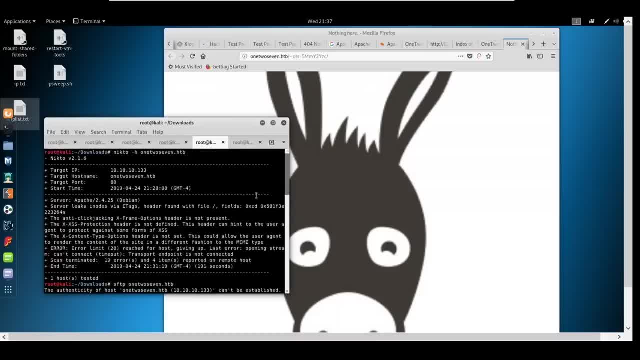 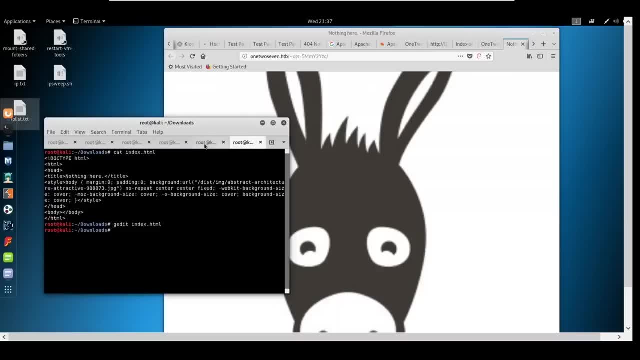 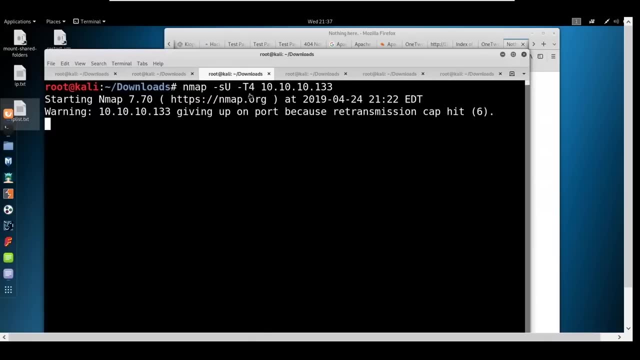 We could also look That got very capture the flag very quick. Unfortunately, I didn't want to go that route, But the old hack the box Heath kicked in and started diving down that route. We would wait for the UDP to come back as well. 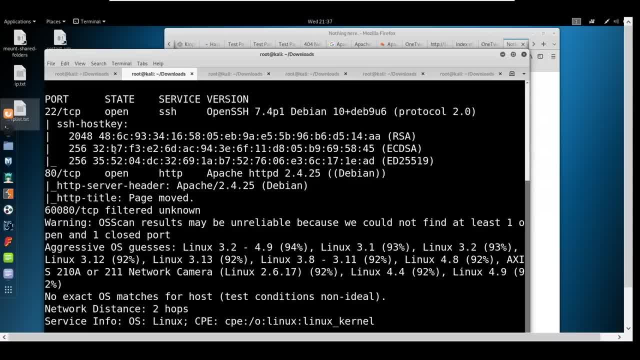 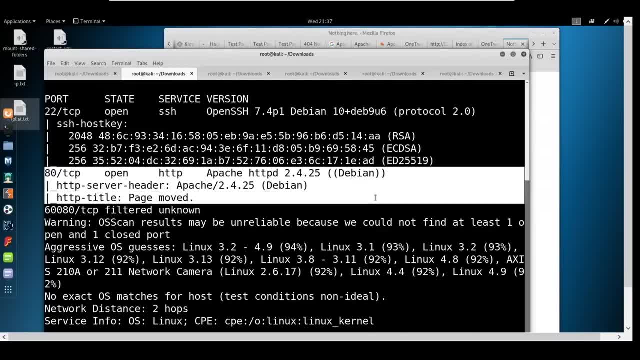 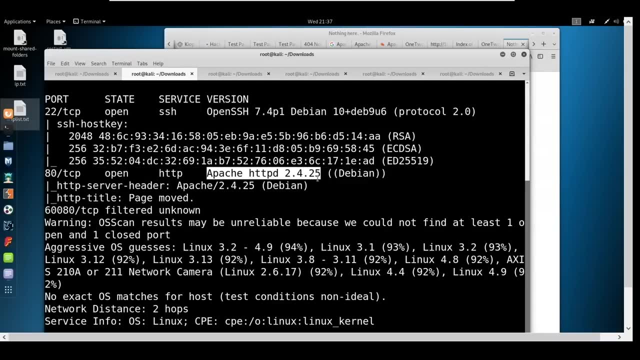 We're at 88.3.. So we'd want to see what's open over there, But we've pretty much pieced together that we've got access to upload and modify a web page via This Apache. We could do research on Apache 2.4.25 via SearchSploit or via Google. 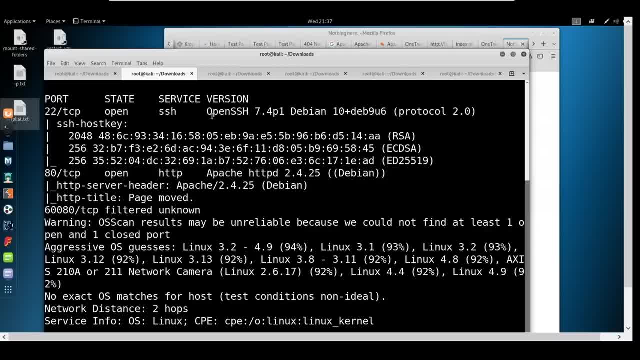 to see what type of exploits are out there. We could do research on OpenSSH 7.4 P1 to see what's out there. It looks like they're running a Debian-based Linux. That's also useful to know- Debian-based on Apache. 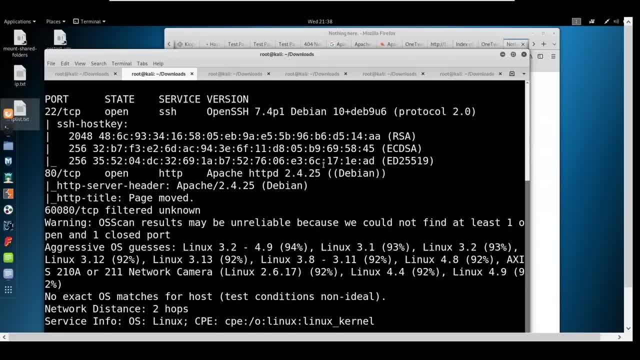 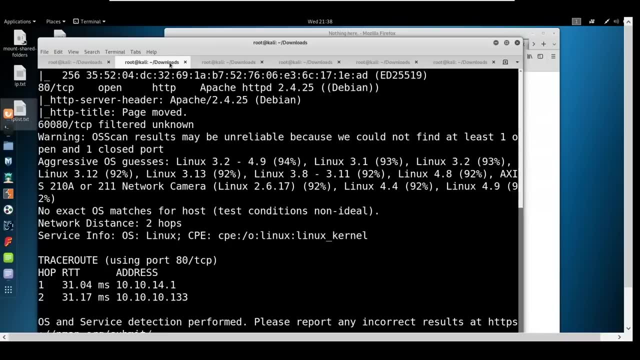 So as much information as we can gather and apply to a later exploit, the better. So I'm going to wrap it up here, as I feel like I can't go any farther. But I see some people are asking about the raffle. 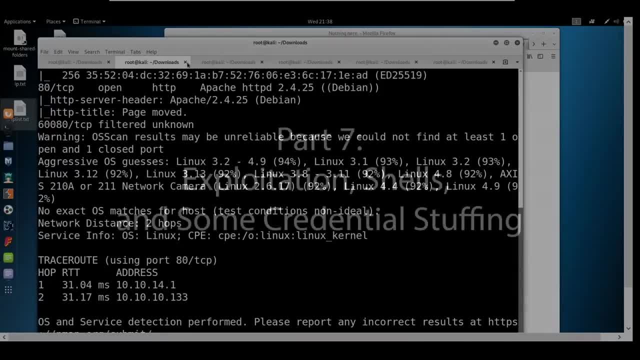 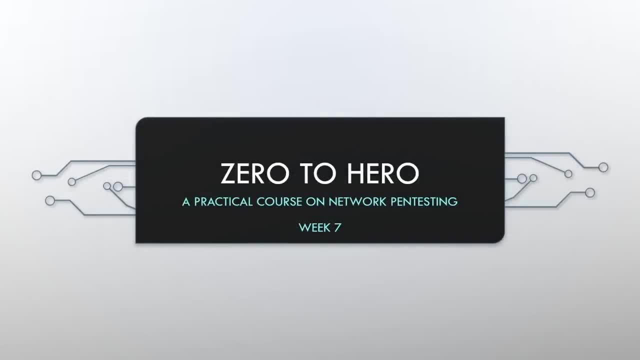 All right, we'll do the raffle. All right, my people, we are in week seven, Week seven, So congratulations. If you've been following along this far, you've made it farther than most. So what are we going to be doing tonight? 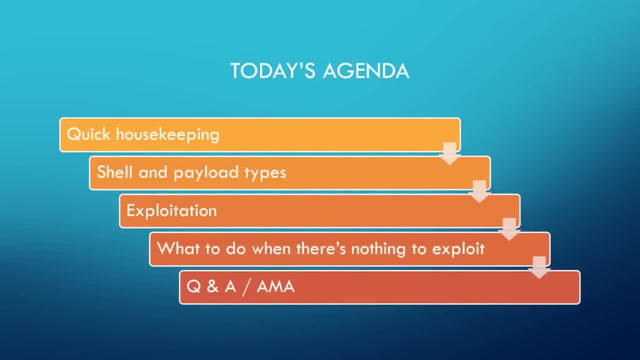 We are going to be doing some quick housekeeping- No more than five minutes. We're going to be doing some shell and payload types. We're going to be talking about exploitation. We're going to talk about what's to do when there is no exploitation. 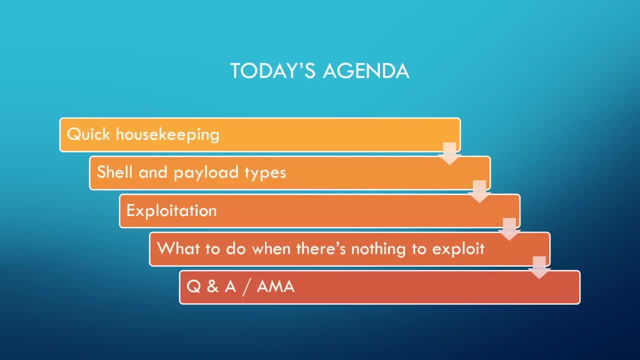 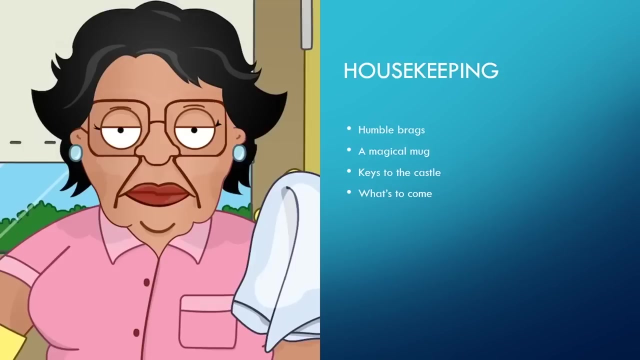 There's nothing to exploit. What can we do? And then, finally, we're going to end with Q&A and AMA. So let's go ahead and go right into the housekeeping. So, first and foremost, humble brags. You may have saw some stuff around my neck. 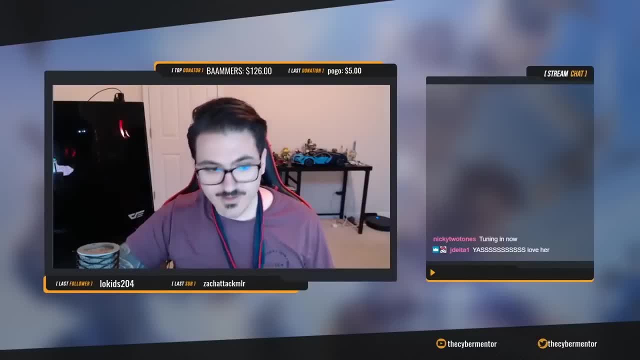 You got to stay humble, guys. This is just me staying humble. So Badge number one: attendance badge. It's actually my wife. Badge number two: Speaker badge. This is all for CarolinaCon. Badge number three: the black badge. 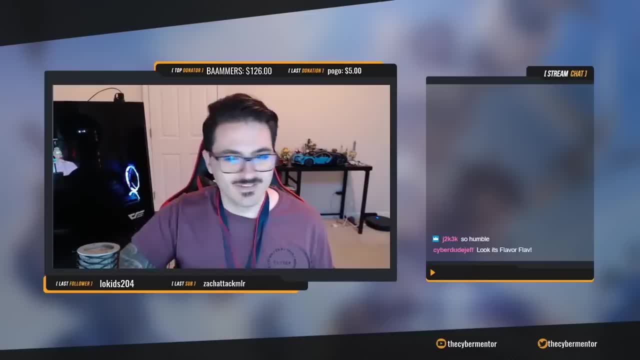 Won the wireless CTF. What's up? Attendance for life. I'm over here like Flavor of Flav. Thank you guys. Again, you have to stay humble, You have to stay humble, But you guys go to cons, come back. 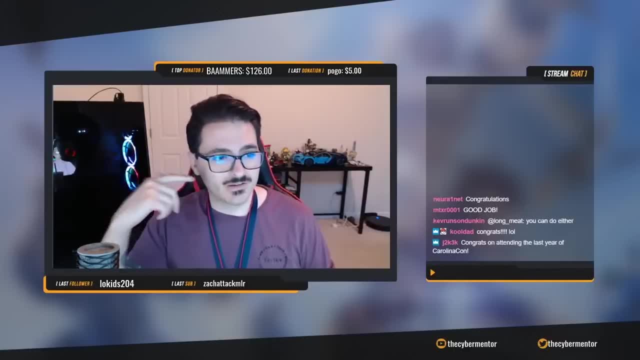 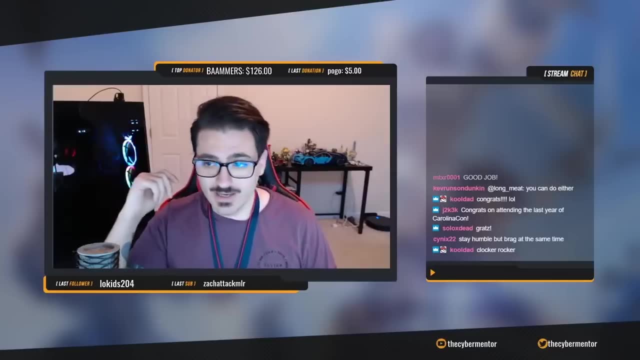 CarolinaCon was awesome. I got to meet some of you guys. Uh, Gray was on my team. Gray won as well, So I mean it was fun meeting some of you guys. Awesome giving a talk. Awesome playing the CTF. 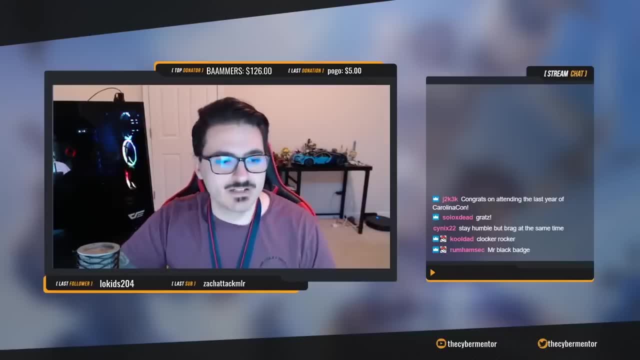 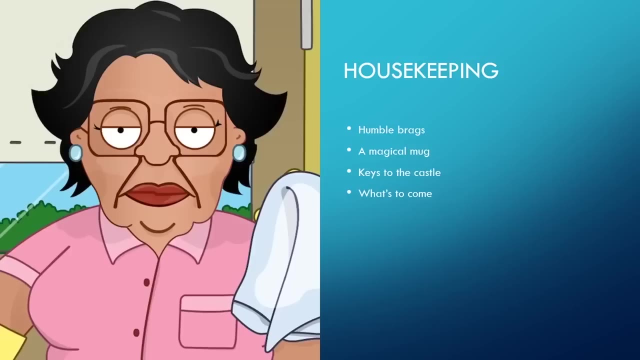 So really cool, And Rumham was there too, So it was really cool, guys. Other than that, you guys have asked for a magical, magical mug. I have put my ugly mug on an ugly mug, If I ever give out any more mugs. 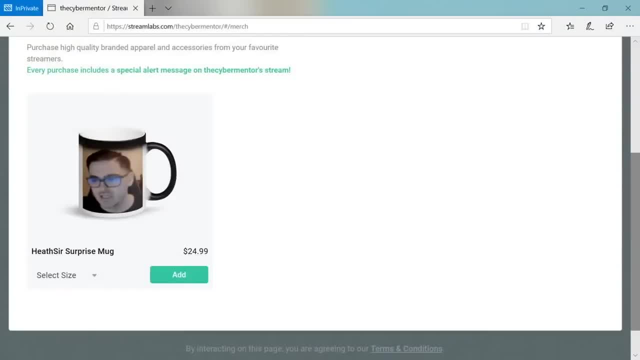 merch than this. please shoot me, because I've sold out. This is your heat, sir mug. It's when it gets hot. It shows my face. You wanted it. This is what it is. No more merch after this, guys. 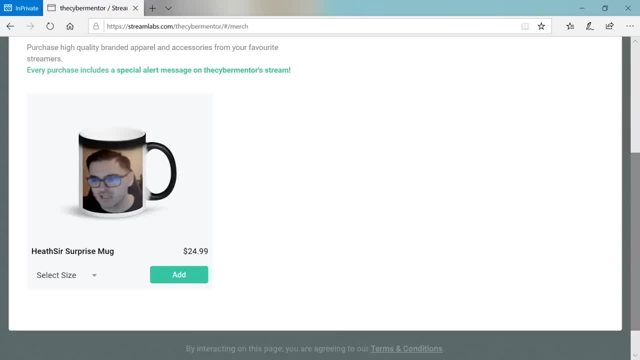 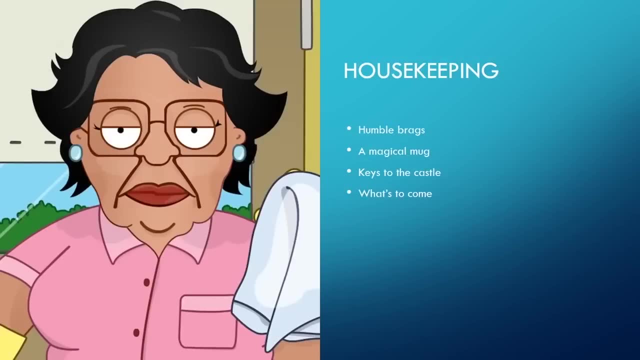 This is pretty much it, So if you want it, there's a link down below. Other than that, please leave me alone about the merch, This is as far as it goes. I did order one. We have had some orders and, yeah, J Delta bought one. 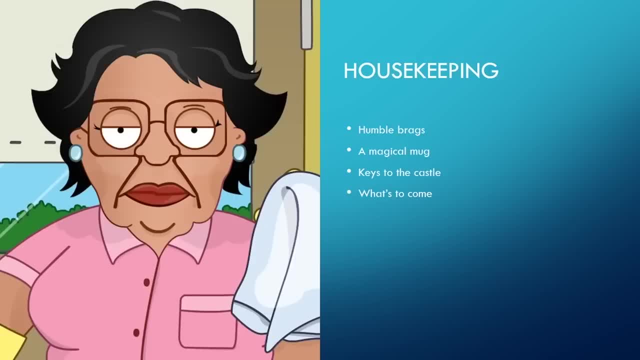 I think it's funny. The prices are insane. Please don't blame me for that either. All right, Keys to the castle. So after tonight, we have been through everything you need to exploit a machine on an external network. With that being said, 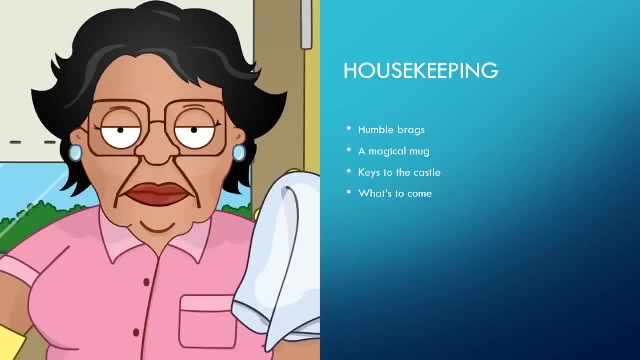 I haven't given you every single tool or tactic that you have out there, but I've given you the methodology, the lesson plan, everything that you would need to do the exploit. Now it's going to be up to you to put in the work on the enumeration. 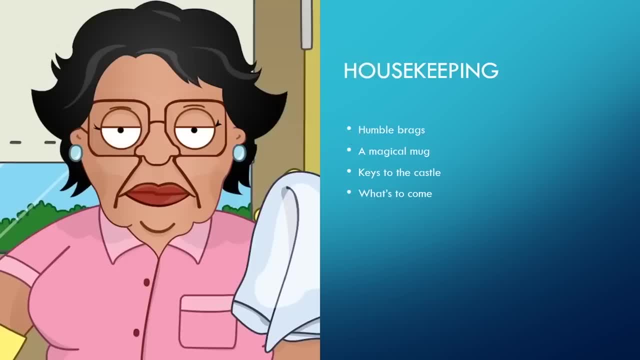 to put in the work, doing research, to finding the right tools and figuring out if things are exploitable. All we're doing tonight is covering some exploits. We're covering some, some of the basics, but I would have full confidence in you guys now going out. 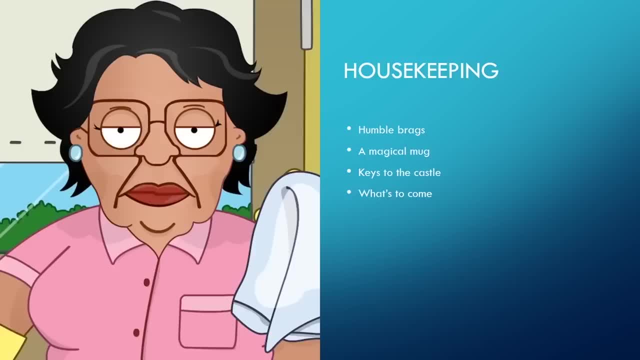 and practicing some capture the flag capturing or practicing some basic level hack the box, practicing some volume hubs, just on the easy side, where we haven't gotten into the the escalation side yet. But you can imagine, as of now you're getting the routes. 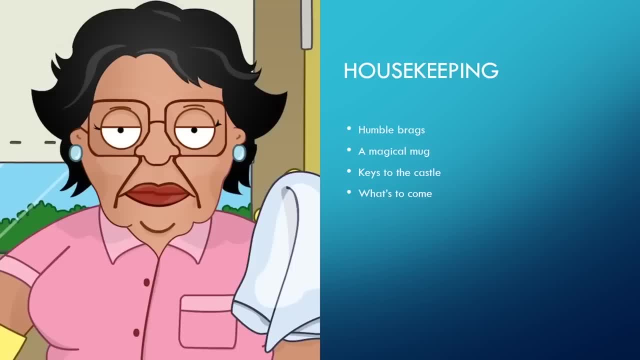 that are just insta wins, and that's good. You have the keys to the castle. You are really far ahead now than where you were seven weeks ago. That's awesome. From here, what's to come? A lot of you have been asking about privilege escalation and 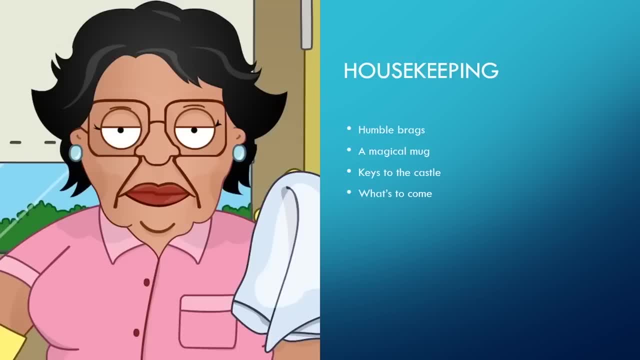 I'm indifferent on privilege escalation, so I can sit there and I can teach you some things and I will show you some concepts. right, I'm not going to Show you the traditional. I'll give you links, I'll send it out, but I'm not going to show you. 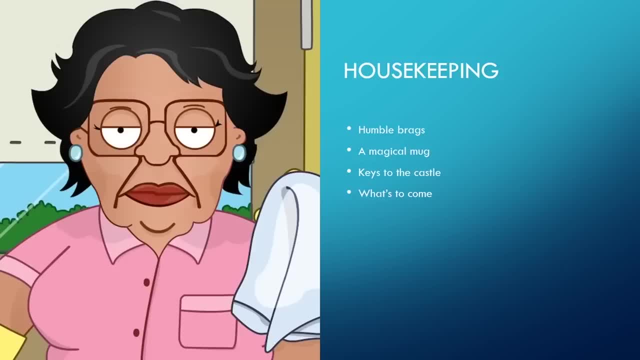 the traditional capture the flag type. That's just not realistic. So what we're going to be doing from here is we're going to be building out an active directory lab. I'm going to be sending out a link to a Windows Server 2016 trial. 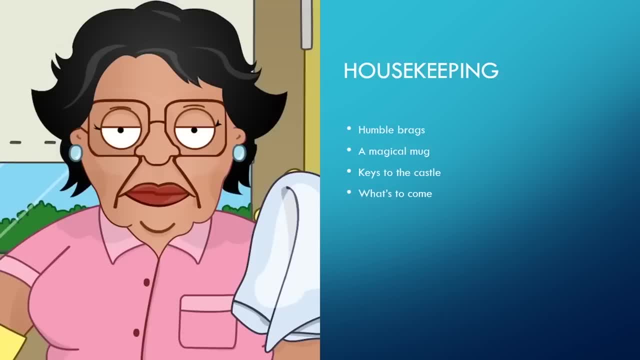 We're going to have like a Windows seven machine and we'll have our victim. That'll be our victim machine And then we'll have our, our Cali machine. We'll be running a three system setup and we're going to start exploiting AD as if we were from the internal side. 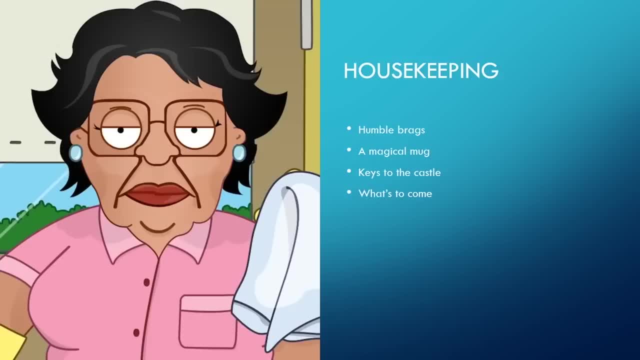 So, with that being said, what we're going to do is we're going to set up vulnerabilities, we're going to exploit them and then we're actually going to cover some of the blue side and and patch it as well, just to make sure that we know what's going on. 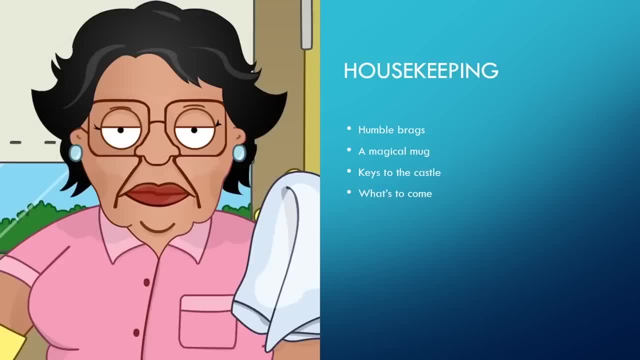 and how we can, how we can take this information and and talk to a blue team, or you're right. So you might say, hey, I found this and here's the solution, And you actually know in the back of your mind how to patch that solution. 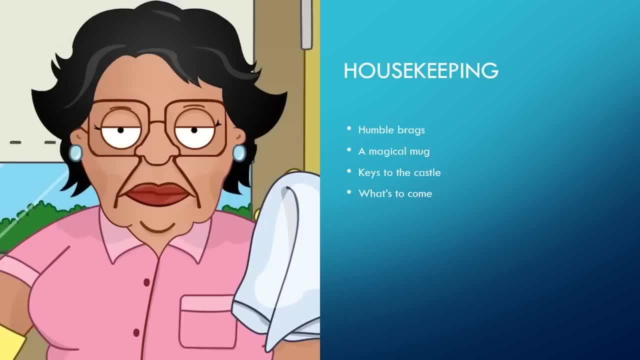 So really good stuff. You're not going to see the traditional privacy because traditional privacy is just not realistic. Traditional privacy to me is talking AD environments. We'll talk about what things to look for. important files and enumeration, Yes, but in terms of you know. 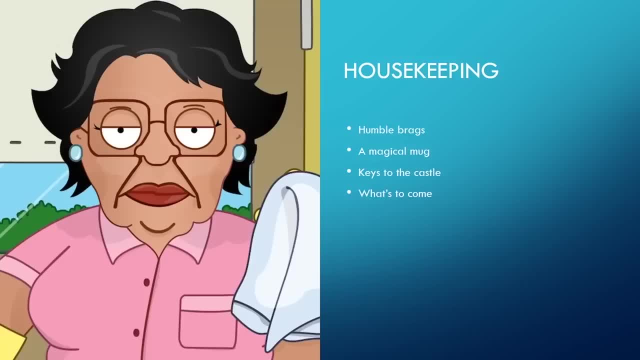 what you see on some of the crazier- hack the box or what you've heard about like the OSCP- most of that's just not realistic. It's cool but it's just not realistic. Hello to all the new people that have come in. 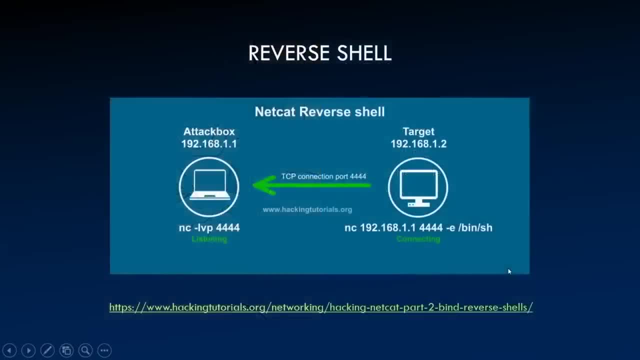 I've seen quite a few of you come in. All right, so let's talk about some shells. We're going to be doing two shell types. really, most commonly, There's a reverse shell, which is by far the most common, and we're going to demonstrate this with Netcat here in a second. 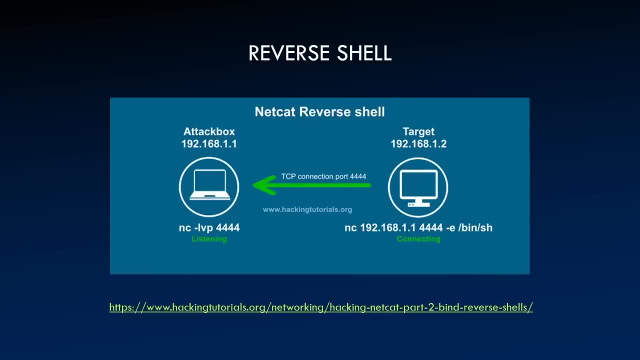 If you've never used Netcat before, it is just basically a port listener or port connector, depending on what you make it do And basically what you're doing. if you see this wonderful diagram that I stole here from hacking tutorials, you could see that 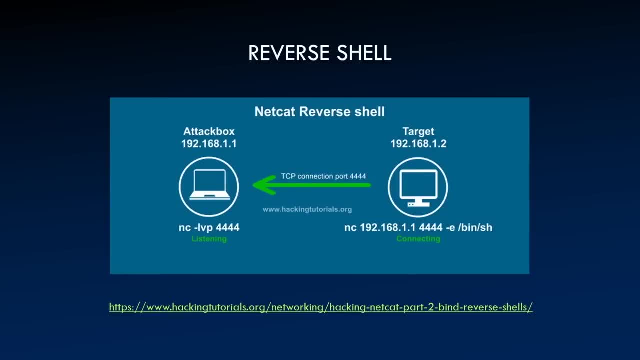 We have a attack box and this is the most common setup. Again, say, attacker IP is the one dot one. Now all they're doing is they're setting up a listener on port four, four, four, four with Netcat, which is NC by default on Kali Linux. 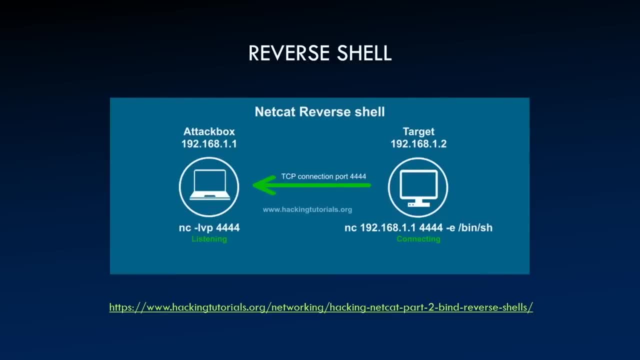 And the target machine is showing the Netcat syntax, And that's fine. That's how we can actually connect. But all you have to do is think about some sort of exploit, which we're going to learn about, or some sort of shell code like you learned about last. 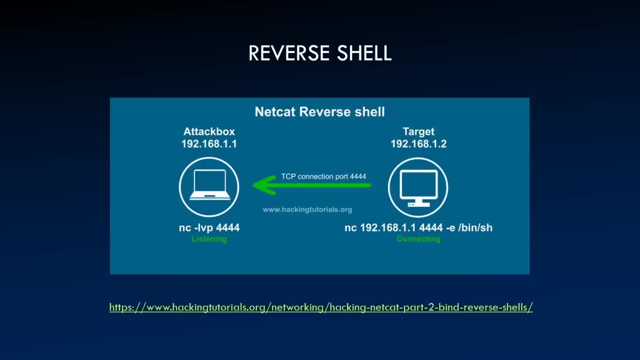 Monday, when Rory was on and Rory was teaching us exploit development, that shell code that you saw, that'll tell the the machine, when it's exploited, to hey connect back to this port, to this IP address. And we're just sitting there listening. 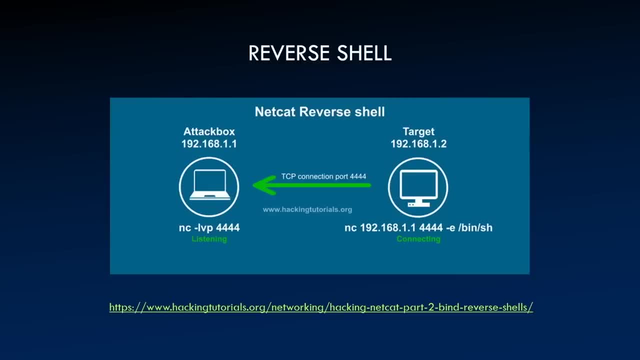 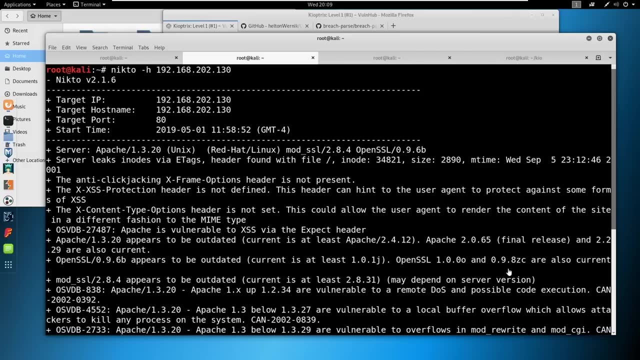 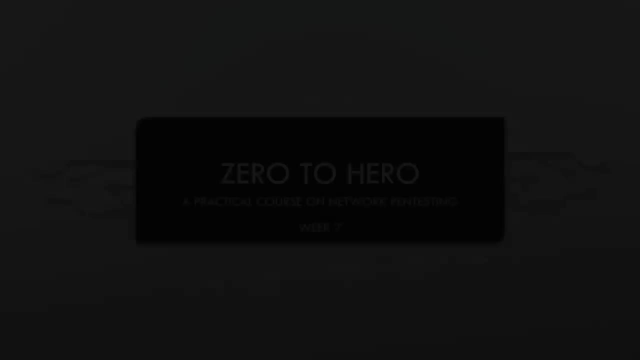 So that's kind of what a reverse shell is. now There's also something called a bind shell, right? So a bind shell is pretty much the opposite, And my PowerPoint presentation just died. That is awesome. One second, OK, bind shell. 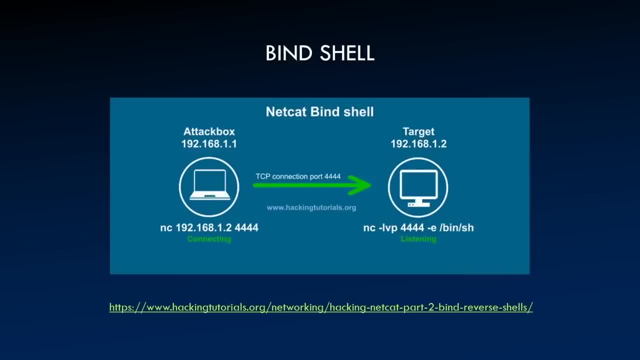 So the bind shell is the opposite. We had a victim connect to the attacker in a sense of a bind shell. We open up a malicious port on the target machine and then we connect to it directly. So it's a little bit different And there are cases where you need one or the other. 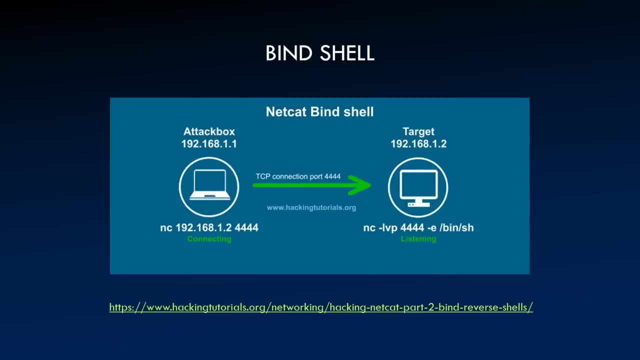 Typically a reverse shell is fine, But imagine that you are on a network, say external pen testing, and you need somebody to connect to you over the Internet. It would almost be easier if you could do a bind shell and connect to them. 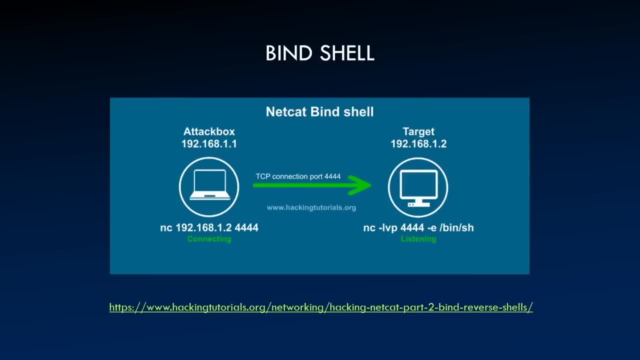 because to get them to connect back to you you have to open up a port on your router, do a port forward and send it to your attacking machine. Now, if you do a bind shell, you pretty much just connect to them directly. 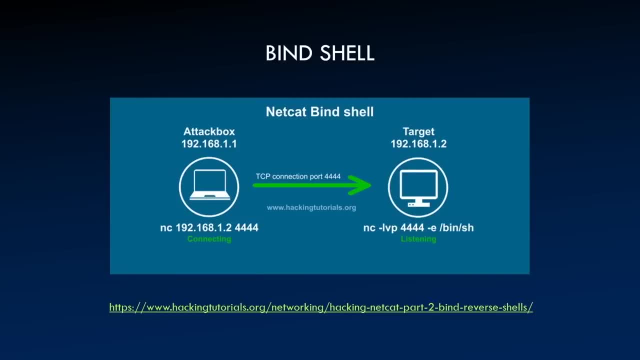 Not saying that you couldn't, but I couldn't do the reverse shell, but the bind shell is sometimes easier. Also, sometimes the reverse shell just doesn't work, So we'll have to try a bind shell. So tonight you're going to see an instance of where a shell doesn't work. 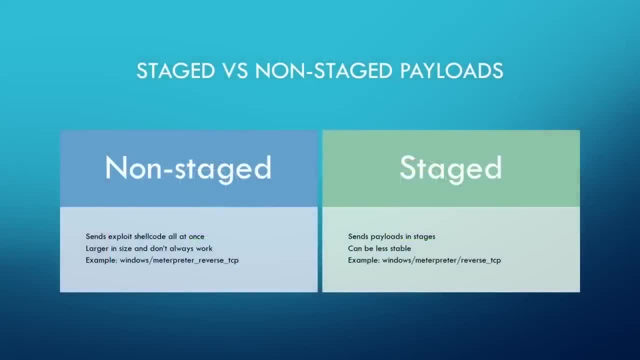 And that actually is going to bring us into the talks of stage versus non-staged payloads. So we have two types of payloads you're going to see And one is non-staged. so basically that's going to send exploit shell code all at once. 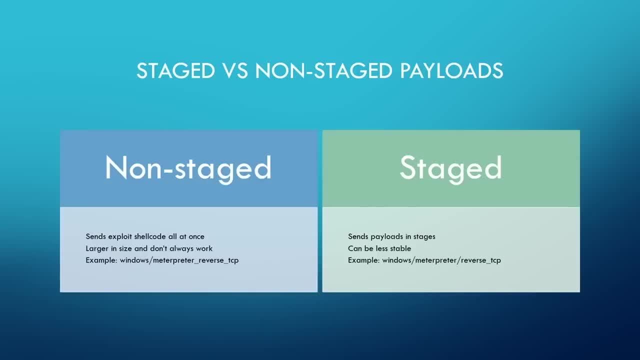 There's no staging to it. It's a little bit larger in size and it doesn't always work. because of that large size Can't always get the payload across. Now, if you see- and we're going to take a look at this later- 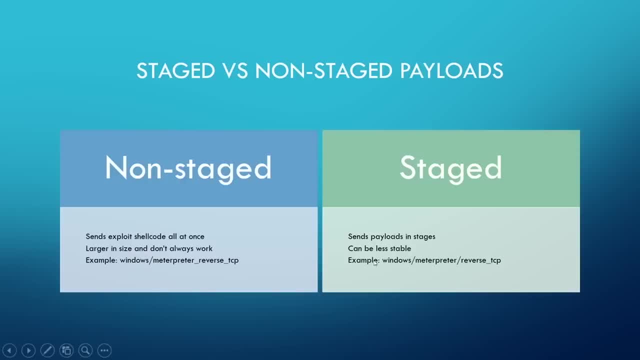 you'll see it more in depth, but if you look at the example over here, you see where it says Windows. it has this slash and then it says meterpreter underscore- reverse underscore- TCP. This is a reverse shell in Meterpreter, a reverse TCP shell. 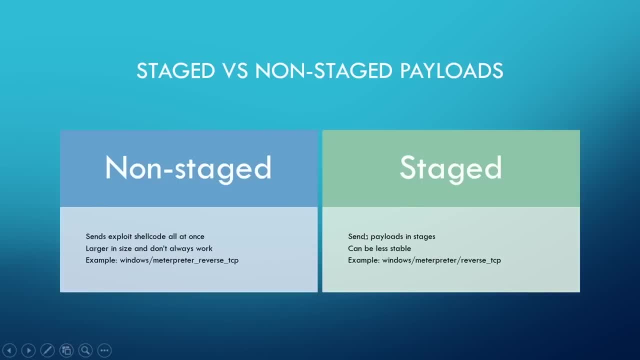 If we look at staged, staged sends the payload in stages, so it's opposite right, But it can be less stable because it's sending things over in stages. If we look at a staged payload, it looks a little bit different Where there was an underscore over here. 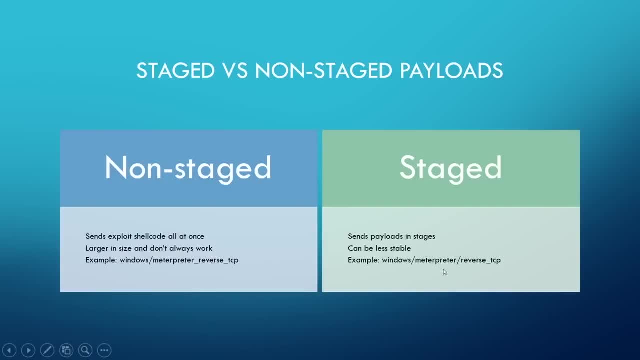 now there is a forward slash, So Windows forward slash, Meterpreter, forward slash, reverse underscore, TCP. So a little bit different there. Now, before we get into tonight's lesson, I am going to show you a brief example of our bind shell. 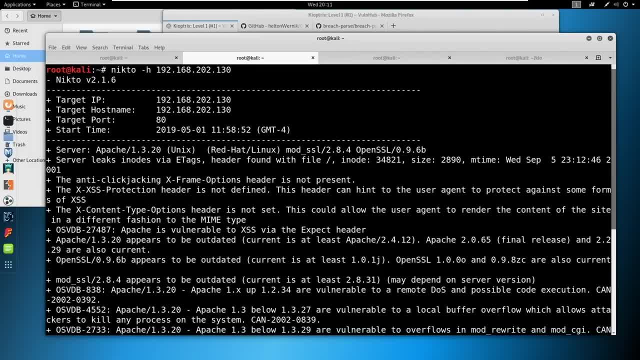 So I'll show you how to use Netcat and we'll do a quick bind shell. You might not be able to do this, You might just have to follow along. So let's play victim and let's play attacker. So on this, let's play this machine, being the victim. 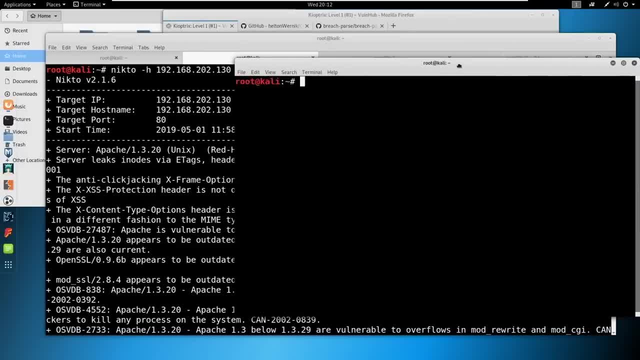 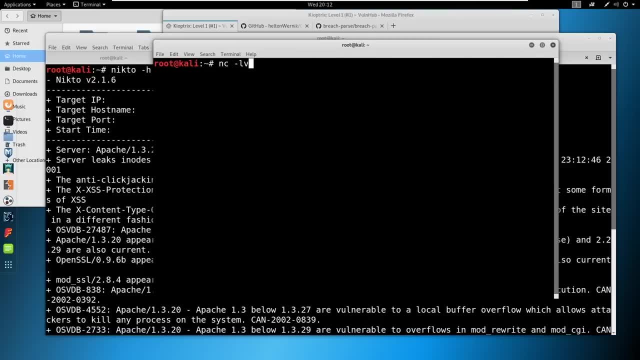 Let me open a new window here. And the victim in a bind shell has been exploited And let's just say that the shell code opened up a port on 4445.. And it's a Linux machine, so it opened up a bash terminal. 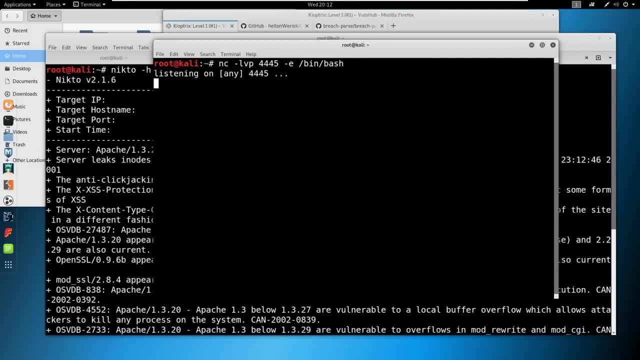 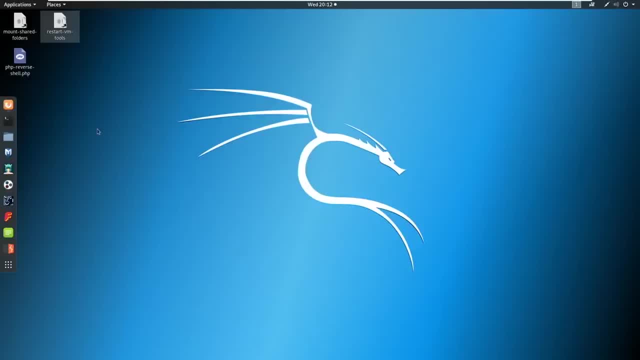 or it's going to open up a bash terminal when somebody connects to it. Now I've got my fancy other stuff over here, right, My real pen test machine. Let's open this one up And let's just say, okay, I'm the attacker. 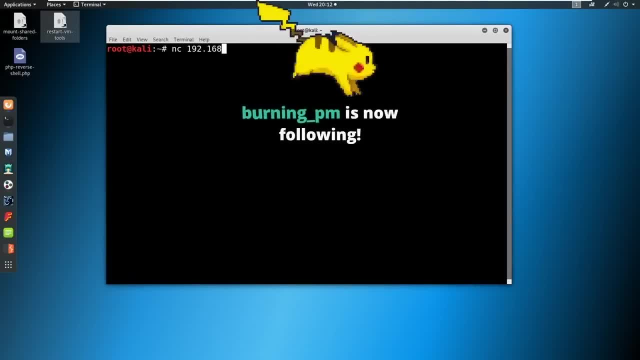 I'm making a bind connection. All I need to do is reach out to that machine, which I think is on 129.. We'll see And try to connect over 4445.. Nothing's happening visually, but let's take a look over here. 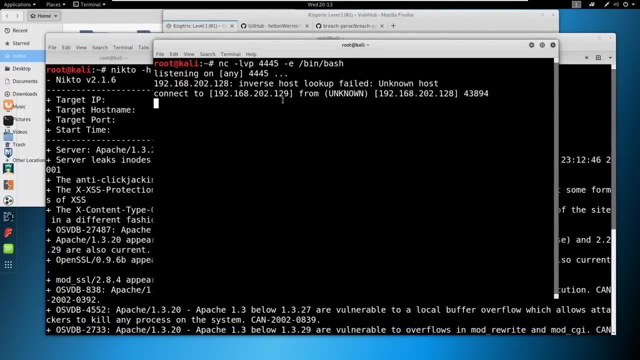 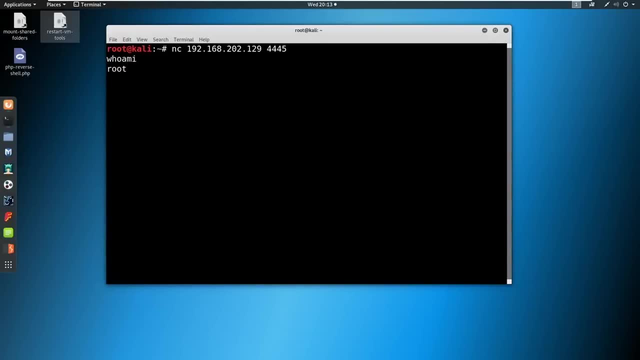 Okay, so we did get a connection here And, And you see, we connected to 129 from 128.. It opened up this port And let's see here, Let's say, if we say, who am I? There's actually a shell here. 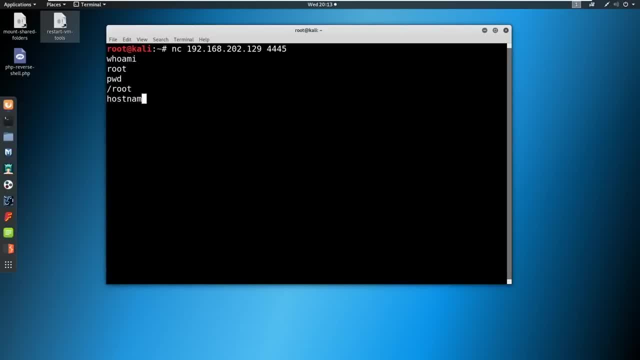 Present working directory. We're in root Host name. It's Kali, So this was an example of a bind connection. Now what you need to pay attention to is the syntax. If you're connecting, all we need is Netcat, the IP address. 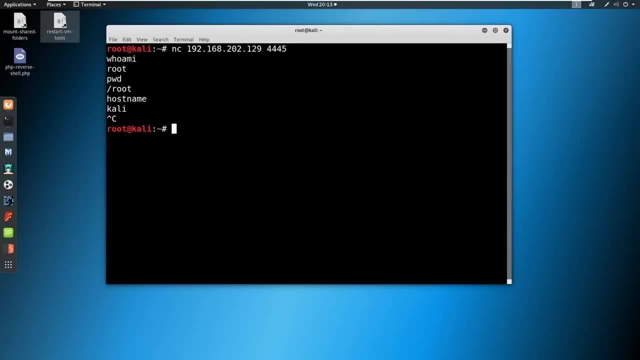 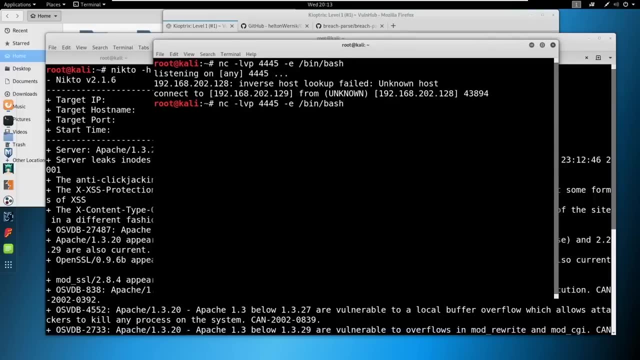 and the port we want to connect to. If you're listening, let's go back to my other machine- And this is typical listening: Just Netcat TAC LVP and then the port you want to listen on. So I use 4445.. 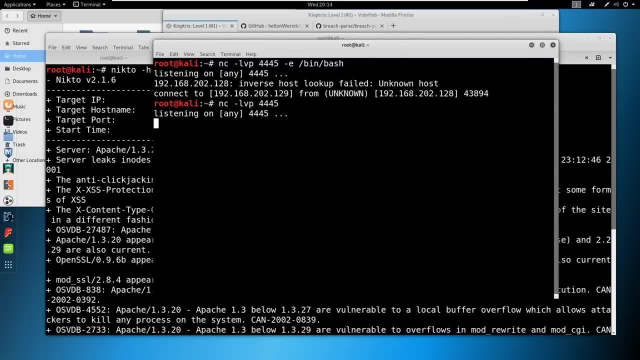 You see a lot of times like Metasploit's 4444.. If you start getting traffic, you might use 443 or 80 to try to bypass filtering, Because a lot of AVs block port 4444, or the firewall will block it. 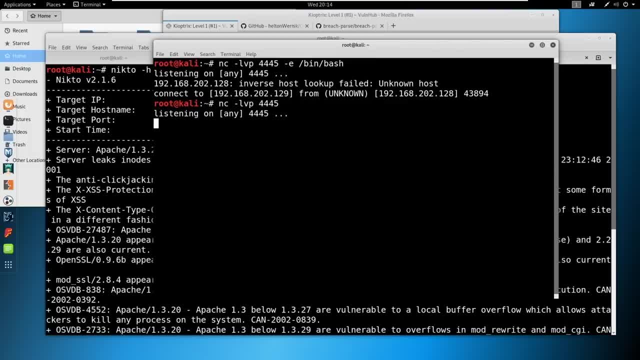 So starting to become well known on that end. You will see this a lot when it comes to running exploits, when it comes to doing capture the flag. You don't see it as much in the pen testing realm unless you have to have it called back to you. 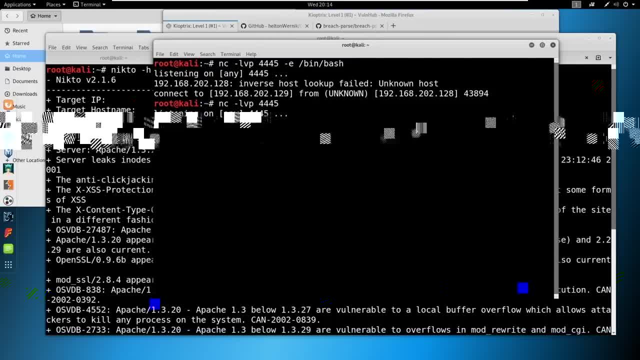 Not saying I don't use it, but you don't see it as much. You're going to see it way more when you're dealing with capture the flag stuff and hack the box or OICP. But very, very important to know how to spin up a quick listener. 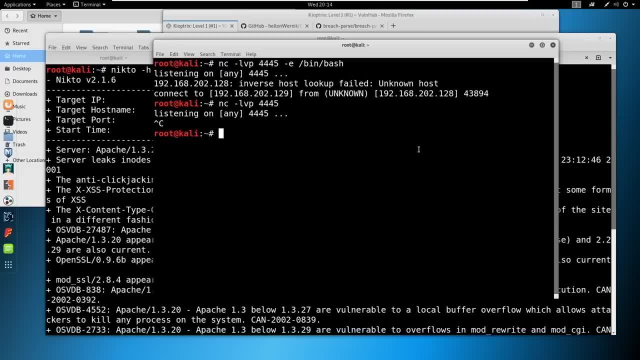 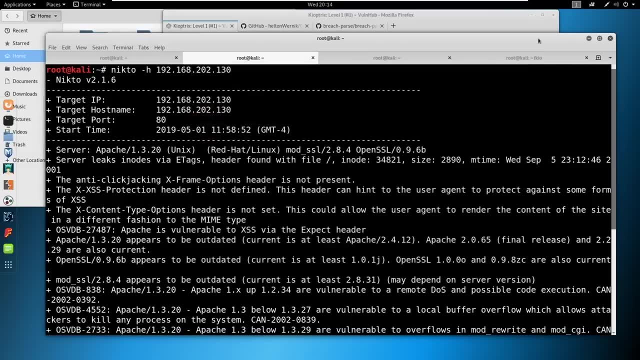 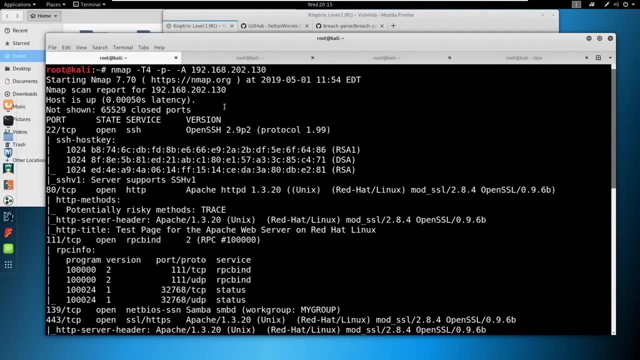 All right, So today is going to be a continuation of last week. Let me go ahead and close this out. And last week we had our scanning lesson, So we did a little bit of mApp, We did a little bit of Nessus. 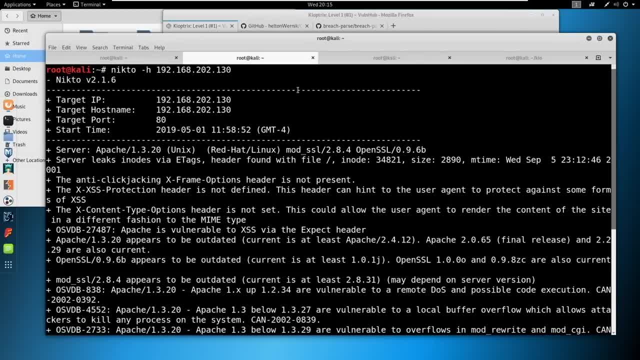 We talked about Nikto, We talked about some other tools, right, And what we found was there were some likely vulnerabilities. One of them was this: Apache mod SSL- open SSL. This line kept coming up over and over and over again, right. 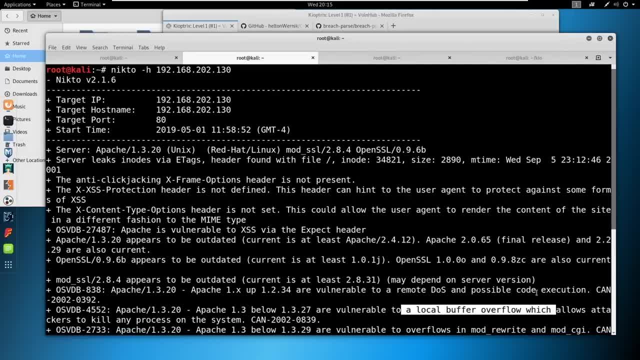 You see it down here. you see a local buffer overflow attack, You see a denial of service, So that one just kept coming up. And we saw it when we Googled it, that it was coming up. We searched for it, It kept coming up. 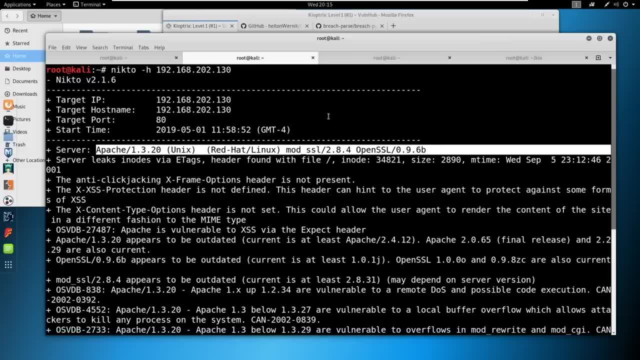 The other one was a SMB type exploit. So today we're going to use Metasploit to exploit one of those And then we're going to use, we're going to do some downloading and compiling off the web and perform another exploit. So you're going to get to see how Metasploit works. 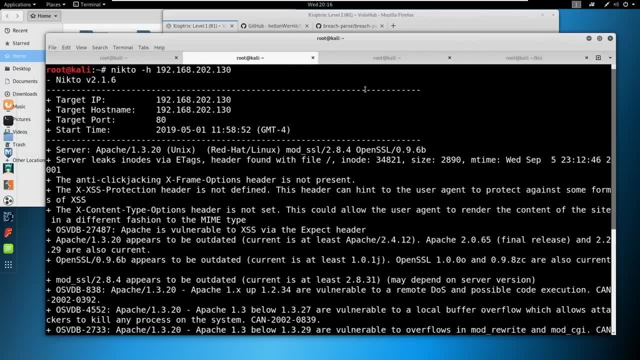 And you're going to get to see how it works for just downloading and compiling something like off of exploit DB or off of GitHub. So what we're not going to do today is we're not going to be working with any type of advanced shells. 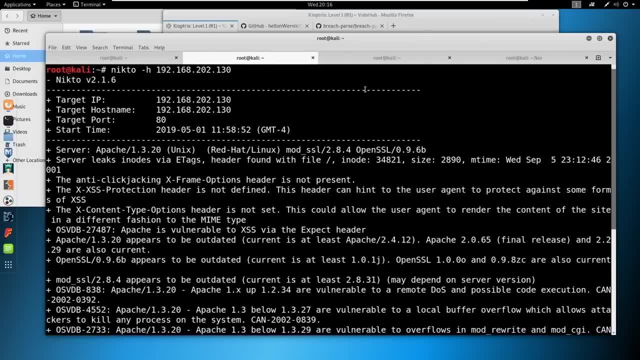 We're going to talk a little bit about payloads when we get into it again, because one of our payloads is not going to work. But what we're going to save is we're going to save everything for when we get into the AD portion. 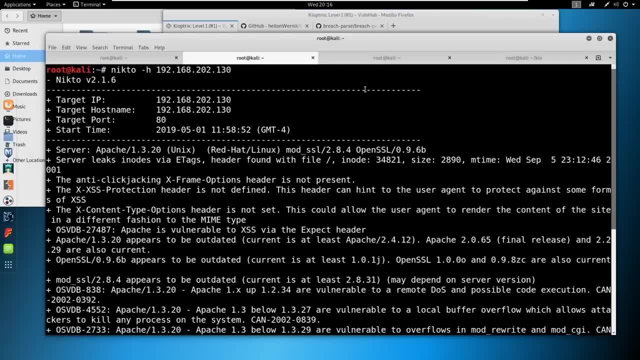 That's going to be the meat of this course. So right now we're all methodology, a little bit of exploitation, And then we're going to get into that exploitation. next week, that post exploitation, We're going to get into more advanced shells. 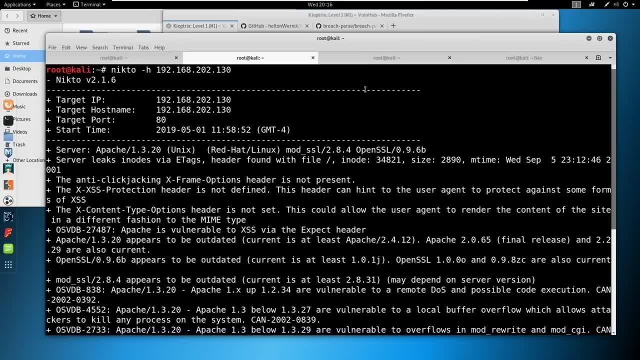 And we're going to keep growing as we have been the past few weeks. So let's start with one of these. Let's go ahead and just start with the more difficult. We'll save the Metasploit one for last. So we've found this Apache 1.3.20.. 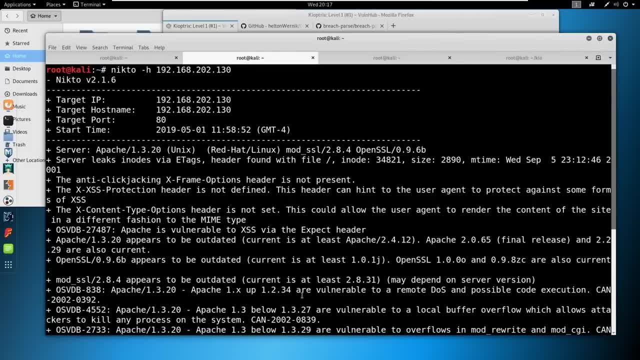 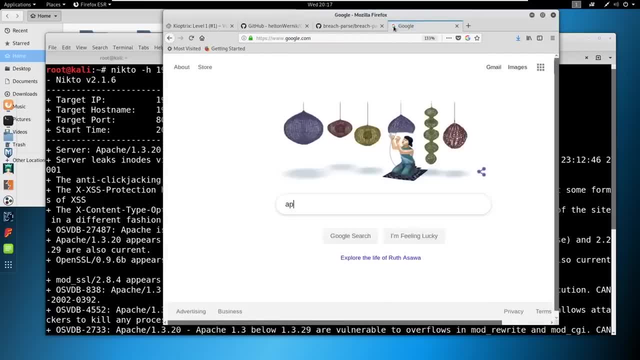 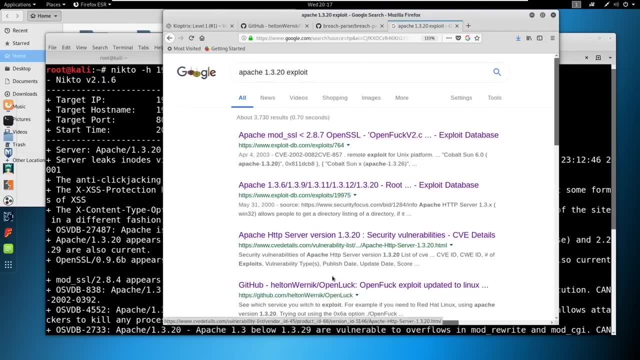 Now, the first thing I would do as a pen tester and if I'm seeing all these things come up, I would go out to Google and I would say, hey, Google, what's Apache 1.3.20 exploit? And you can see- I've looked through some of these things- 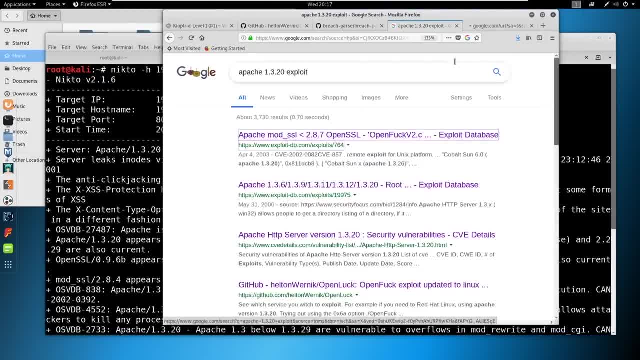 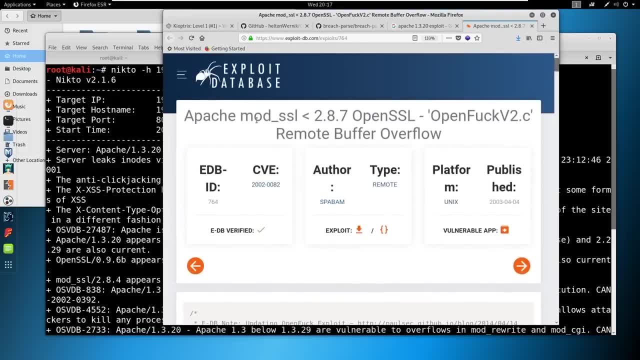 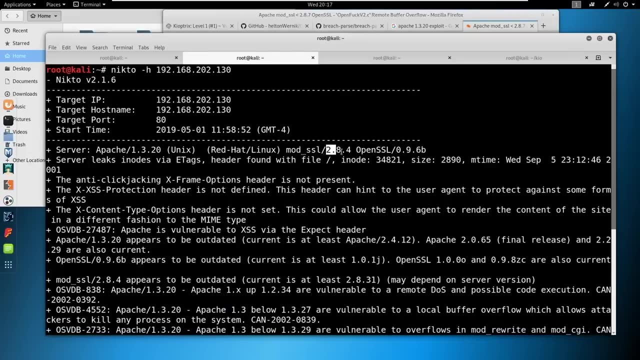 but I would look through it again. So this one- and we talked about this one last week- this OpenFuck, So it's Apache, Mod SSL and the Mod SSL has to be less than 2.8.7.. We match that with 2.8.4.. 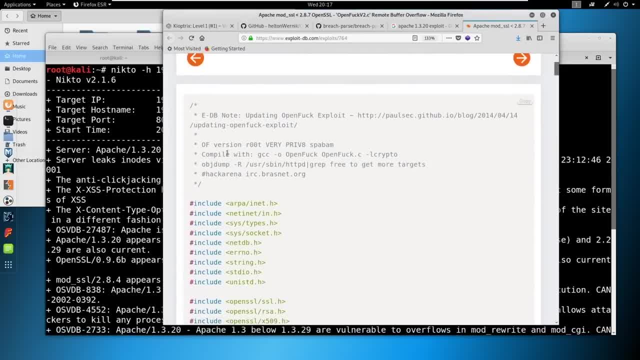 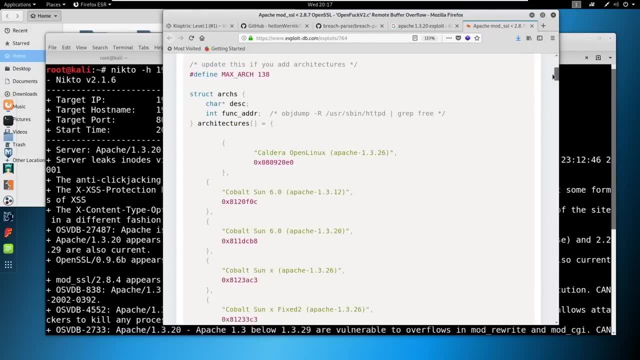 And if we scroll in here, sometimes they give you instructions. They tell you how to compile it And they don't tell you much about it. Sometimes they'll give you a little bit more info. So we would want to do some research on this. 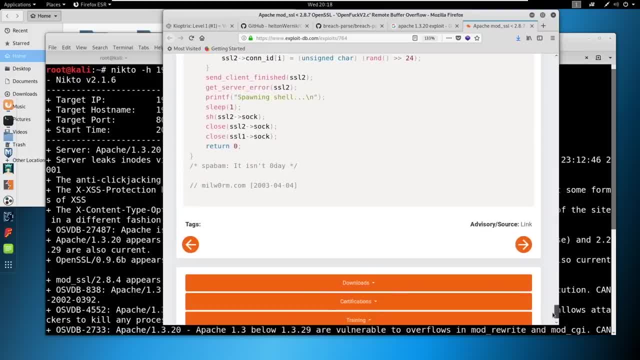 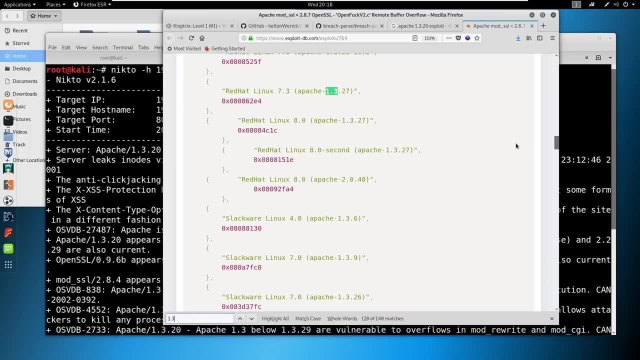 to make sure this is exactly what we're going to be exploiting. But if you come into here and you actually look a little closer, if we just do a page, find 1.3.20, it looks like there's 12 matches. 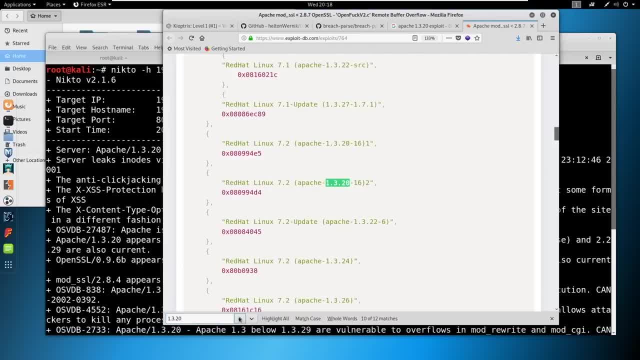 So it looks like the 1.3.20 of Apache is vulnerable And we also know we're on Red Hat. So if we look at Red Hat, you could see that it's got two different versions of Red Hat 7.2, that it's running. 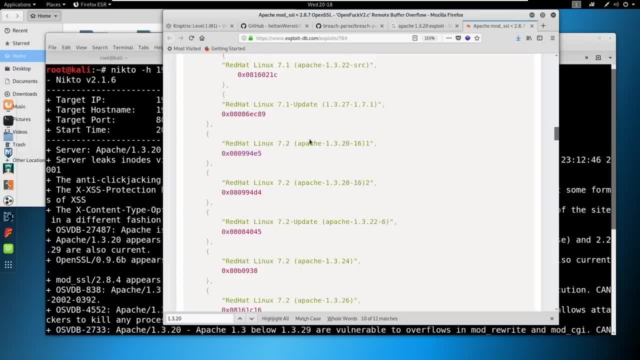 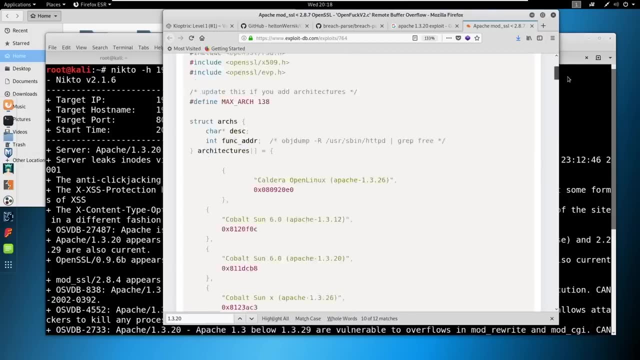 depending on the return address, is what it looks like, And we'll either run number one or number two for that and try to exploit it. So somebody's already going ahead of me, Jeff. This exploit doesn't really work that well, So what we're going to do instead? 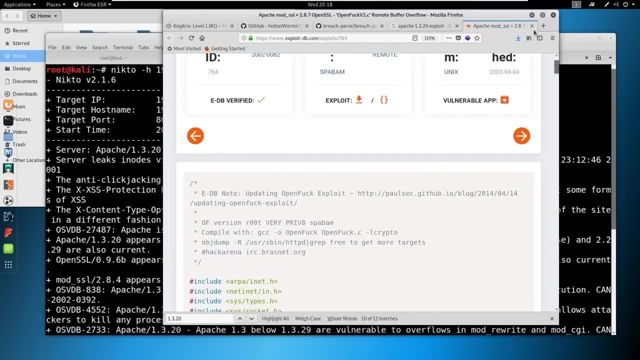 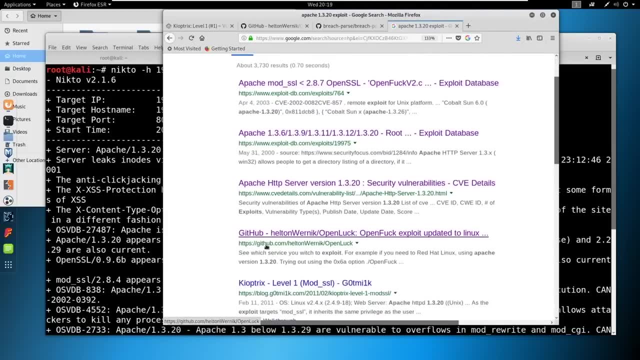 is. we're going to use OpenLuck instead of OpenFuck because we like to have better grammar here. But if you scroll down just four, you see this Helton Wernick or Wernick OpenLuck. I've got it opened right here. 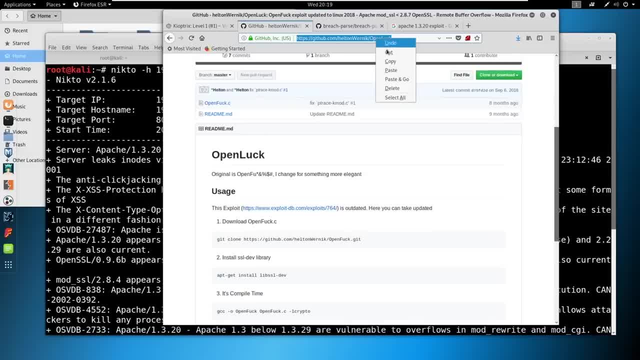 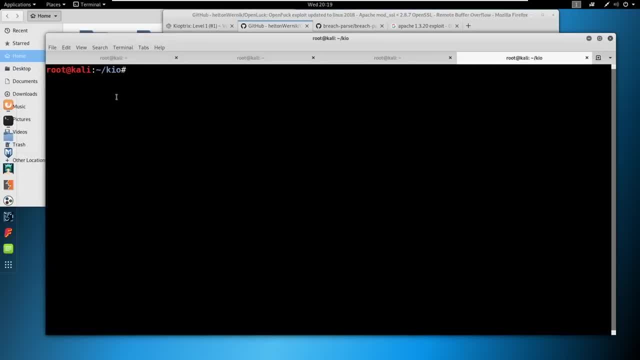 And we're going to use this. So go ahead and just copy this. And I've got a folder just named Keo that I've made and I've compiled this, but we're going to act like I haven't. In fact, I will make a new folder. 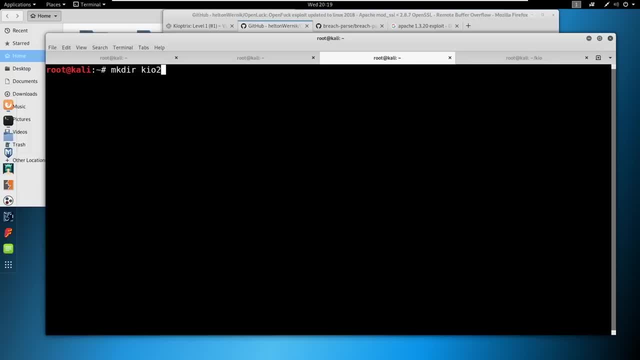 We'll just call it Keo2.. And we're just going to git clone this right. Keo is short for Keoptrics. Okay, so we cloned the OpenLuck. Yes, I do have my OSCP. We cloned the OpenLuck right. 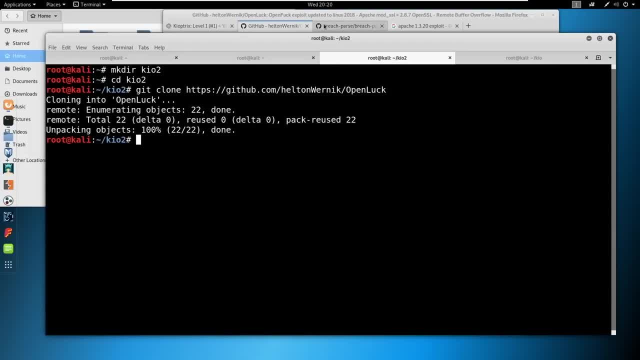 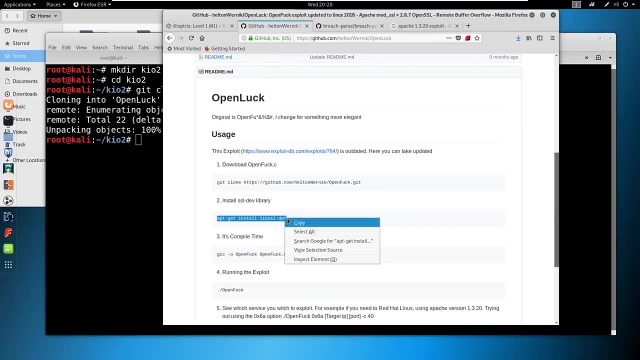 And what we're going to do is we're going to follow the instructions on the page. So it says we've got to clone it, We've got to install this libssl-dev. Go ahead and copy this. I've already got it, but we can try it again. 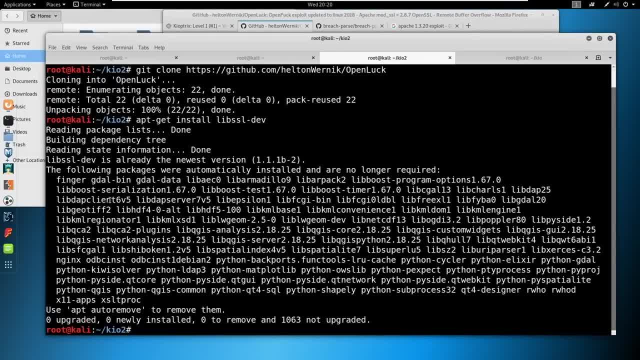 You can see mine's up to date. I will. I'll sit here and wait for you guys just for a second, just so you guys can get this installed, Just in case you are following along. it might take a minute. Hey, Brute505,, are you from New Mexico? 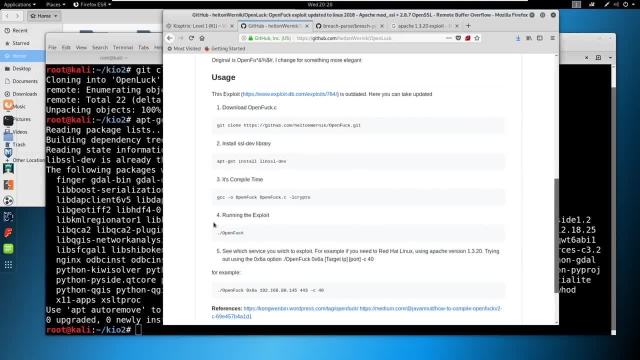 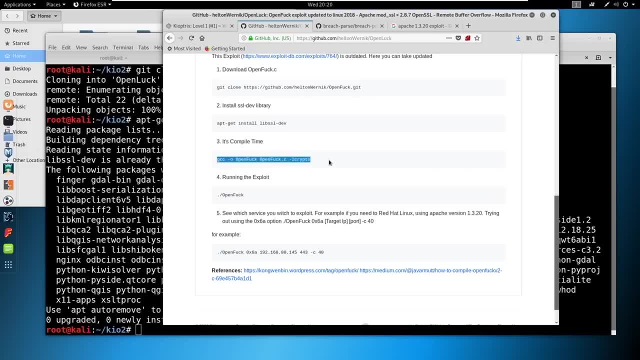 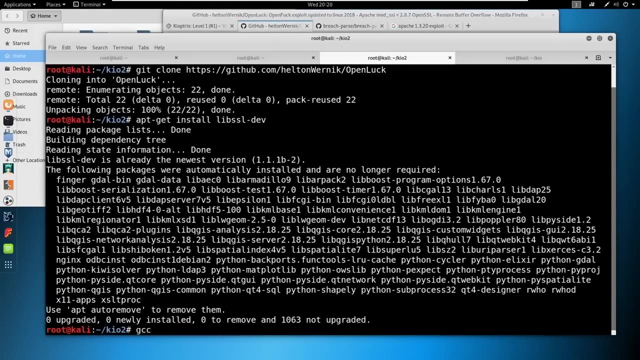 Is that where the 505 comes from, While I give the class 30 seconds here? Oh well, never mind then. All right. So once you have the libssl installed, we're going to compile. So we're going to use a compiler called gcc. 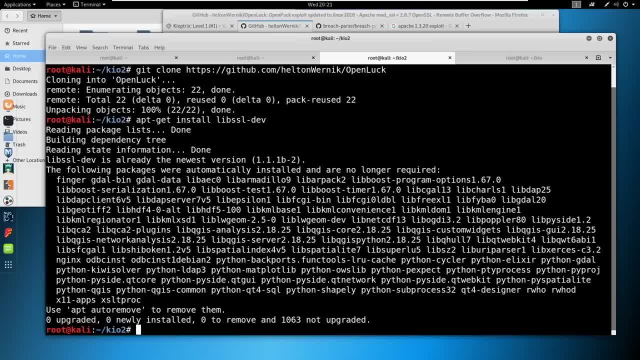 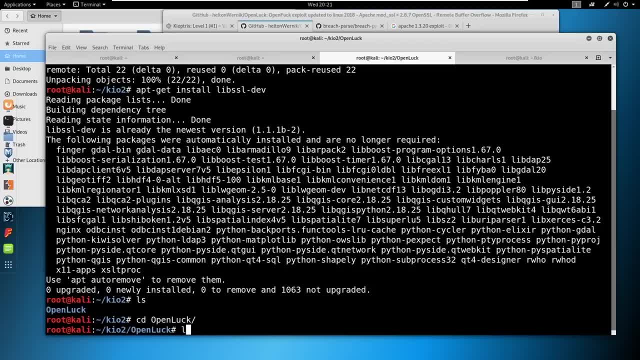 We're going to grab the file we want to compile. I guess I should ls and show you what's in this folder, right? So let's cd openluck ls. Okay, so there's openfuckc and there's the README. 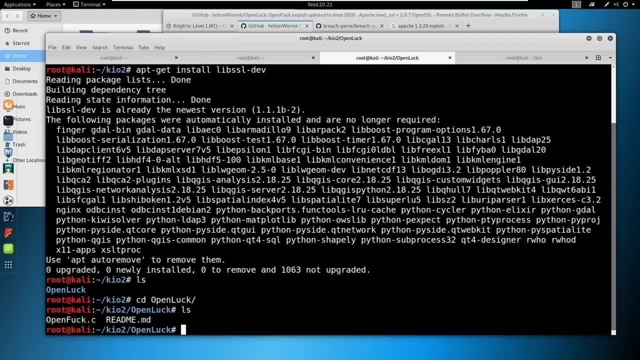 So what we're going to do is we're going to say gcc, Okay, We're going to say openfuck, We're going to do an attack of o and we're just going to name it whatever we want. I'm just going to name it open to be easy. 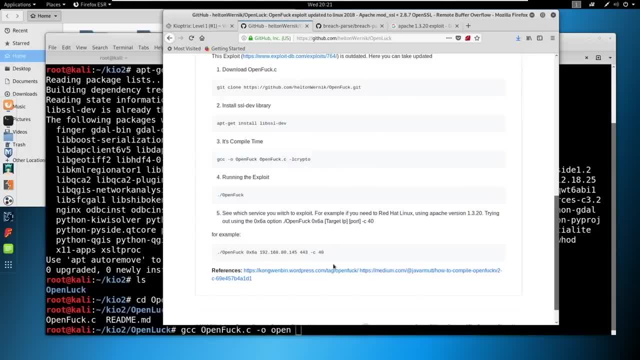 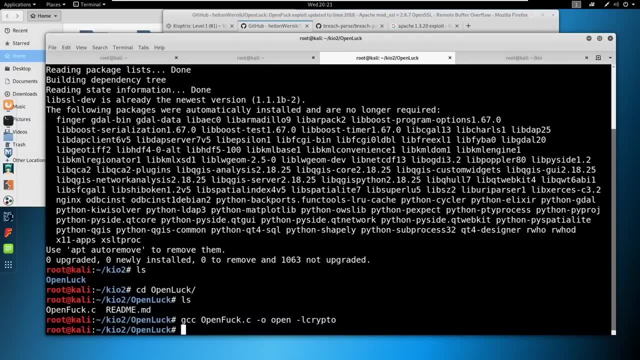 And then there was one more thing. we had one more instruction. It was the "-lcrypto", So we got to type that in as well. Okay, So if we ls, you could see that in green, meaning we have executable permissions on open. 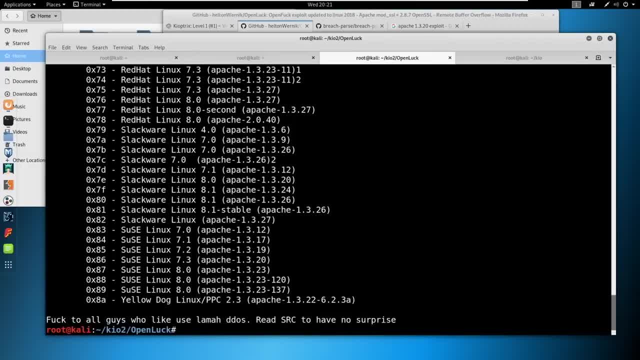 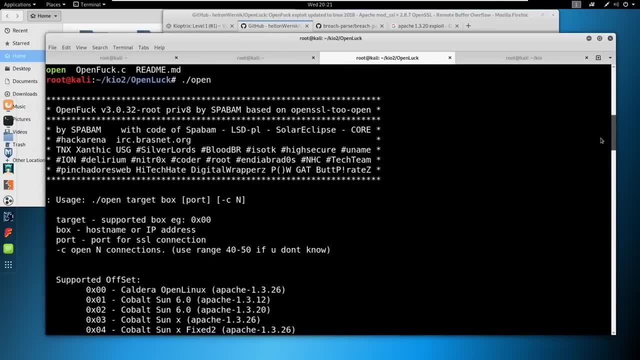 is there. So we just do the dot forward, slash open and it gives us open And it gives us all of the readings here. So the syntax we're going to do dot forward, slash open. We're going to say target box. 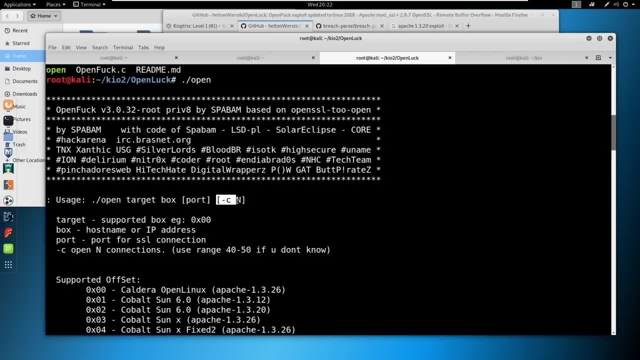 the port and a dash c, So we don't have to declare the port. but we should declare because we're not going to have to run it over SSL. That's fine. We don't know what c is. It says open end connections. 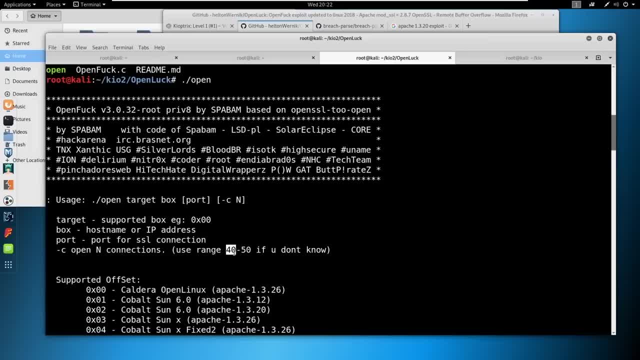 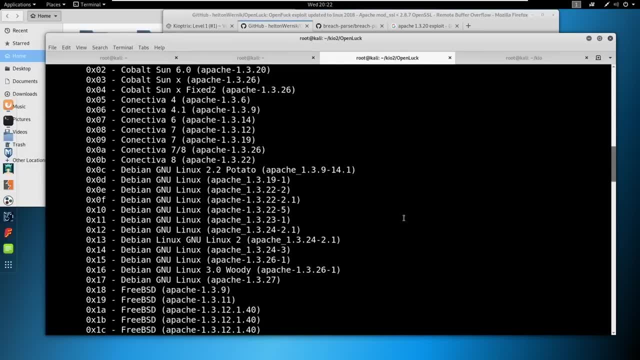 use range 40 to 50.. Okay, So we'll just use 40.. The box is going to be the IP address And then the target is going to be whatever offset. this is in here. So remember we were on 7.2 of Red Hat. 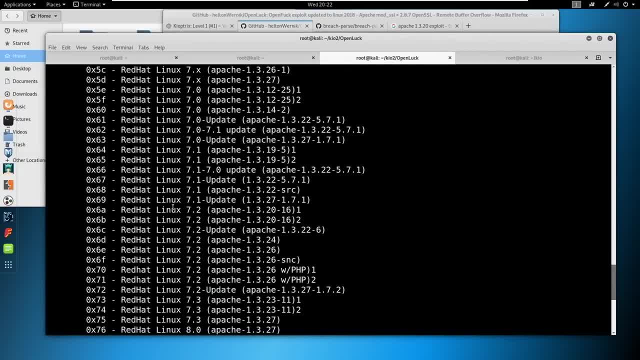 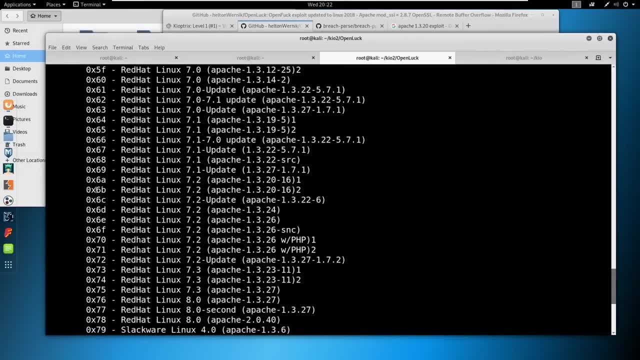 and it was Apache 1.3.20.. So what we have here is we have two options. We've got one or two. I'm going to cheat just a little bit and tell you that it's this guy, the 6B. 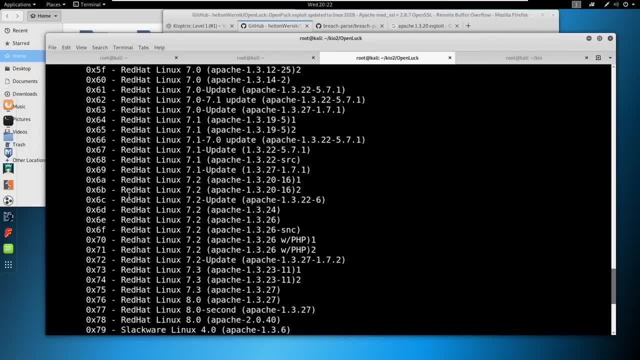 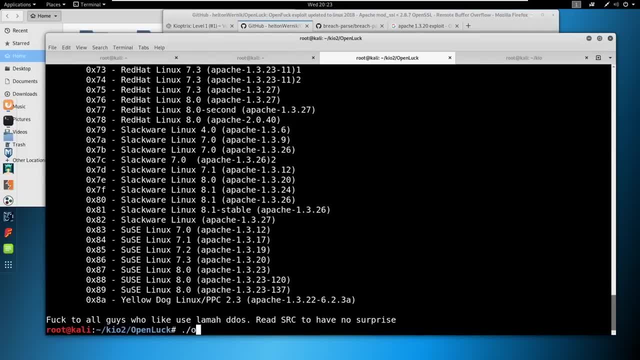 So if we try 6A, it won't work. Then we would just move on to 6B. I'm just going to save us a step and save us some time. So to run the exploit, dot forward, slash open. We're going to say 0x6B. 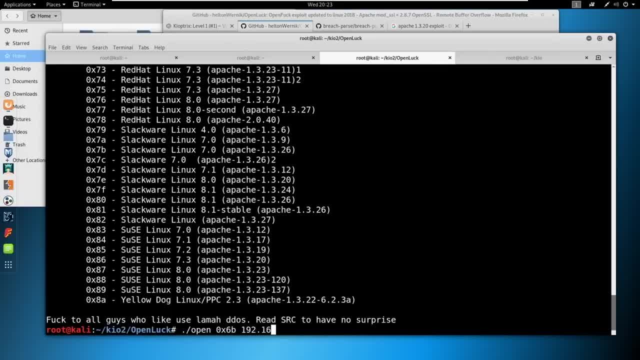 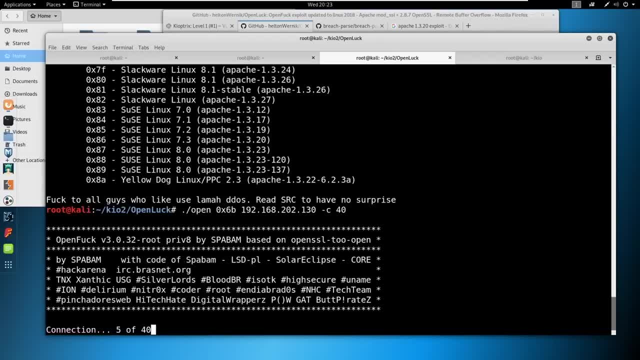 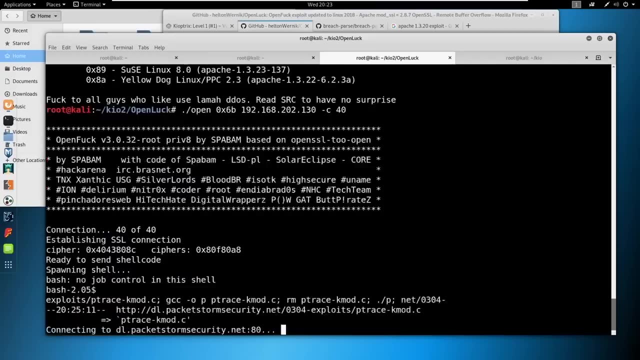 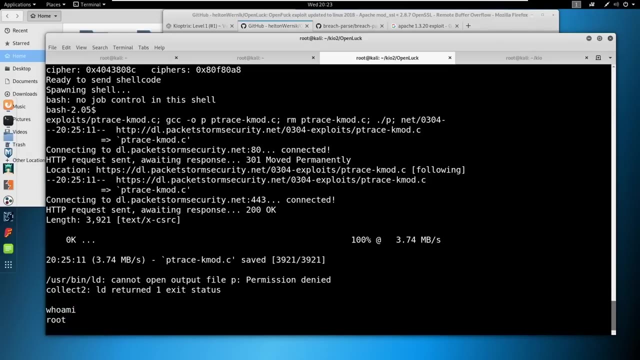 We're going to use the IP address of the machine. we're attacking for Keoptrics And we're going to do the dash c of 40.. I'm going to let that run. See if this gave us a shell back. It sure did. 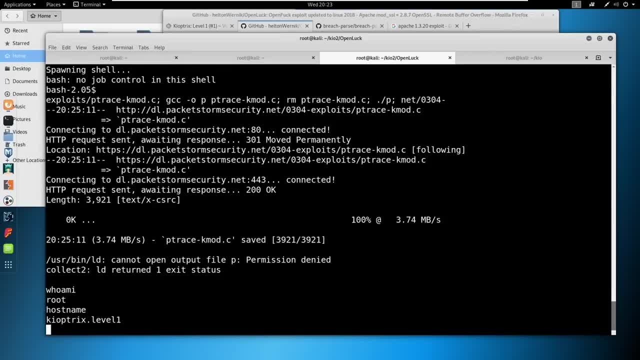 Okay, And we are root on Keoptrics level 1.. So we have just exploited this machine. Now from here there's a numeration that I would do right off the bat And I don't want to go into post exploitation because that's really going to be saved for next week. 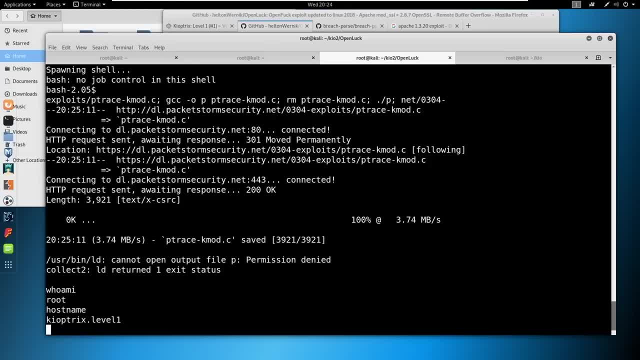 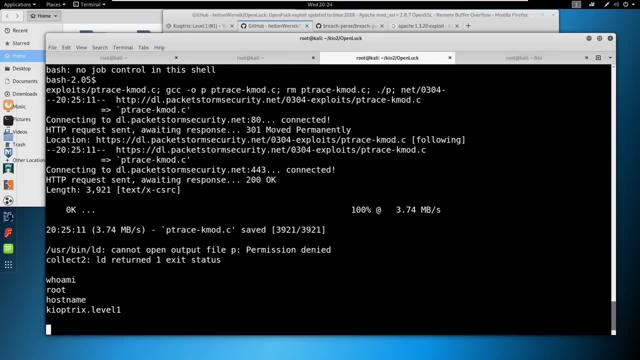 But we should talk about at least a little bit about it, right? So there's some things here that we can do. Me personally, the first few things I like to look at are networking commands And you say: arp dash, a Arp's not found. 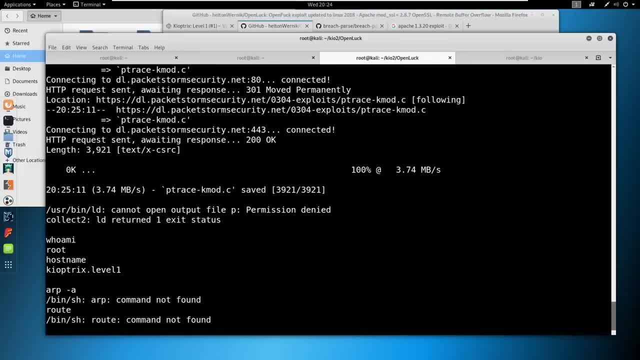 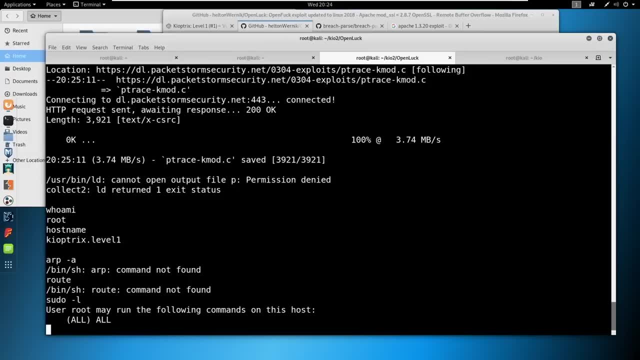 Okay, We say route, Route not found. So sudo dash l. We might not have a great shell here. Sudo worked, So sudo dash l tells us who can run the sudo command while we're root right now. So we're going to run all the commands. 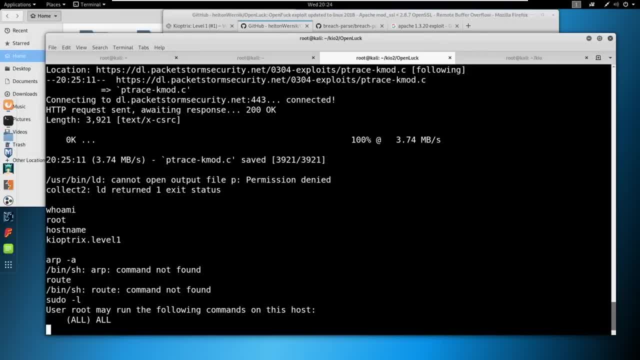 But if you're doing capture the flag type events, this is really good information to know. You might have some sort of tool or command that you can run a sudo that you wouldn't expect, So we could upgrade this to bash. I'm not getting into all that. 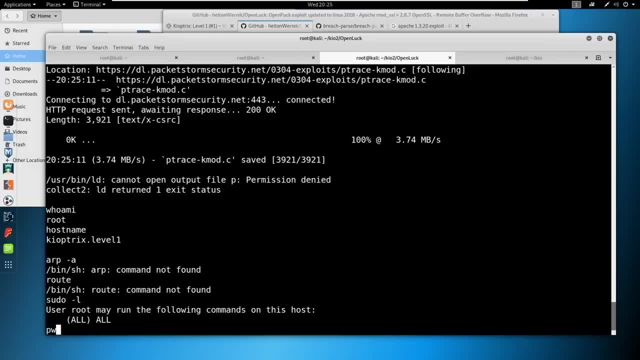 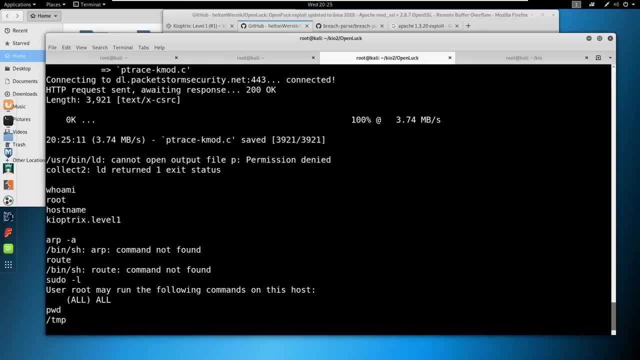 And then so you would want to also see you know what present working directory it puts you into. Okay, It threw you into temp. Can you move around? Can you navigate? Another one I'd look at would be netstat as a networking command. 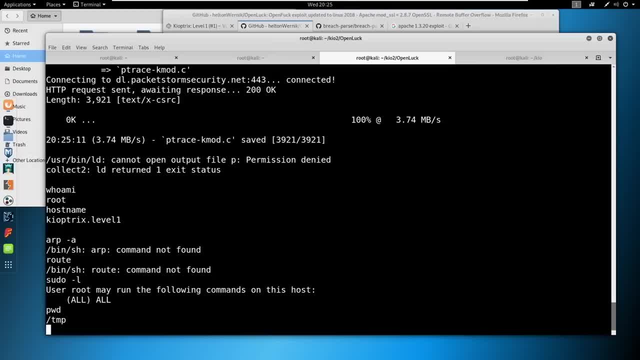 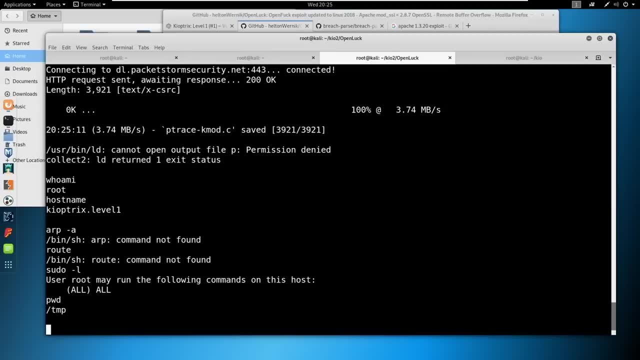 Again, we're going to talk about all this when we move into Windows. It'll be easier to give you the visual. Now the crown jewels are the Etsy password. We could just cat that in the Etsy shadow, right, So you say Etsy shadow. 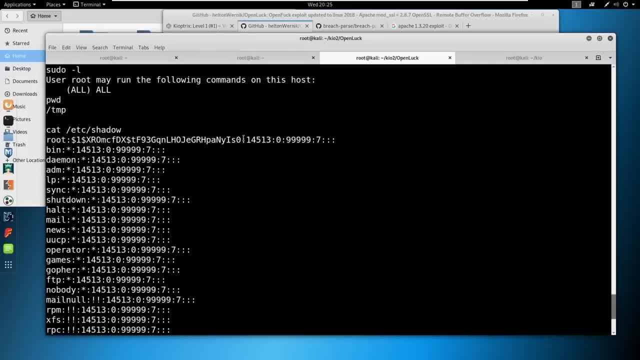 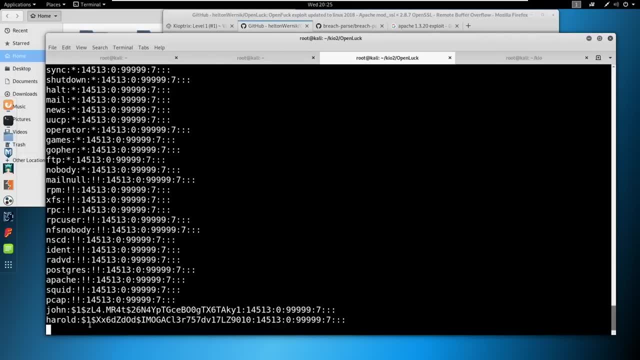 Okay, So there's some users on here. We've got root, We've got root's hash. We've got John and Harold as well, We've got their hashes. So we would take this, We would extract this information. We would also extract the Etsy password. 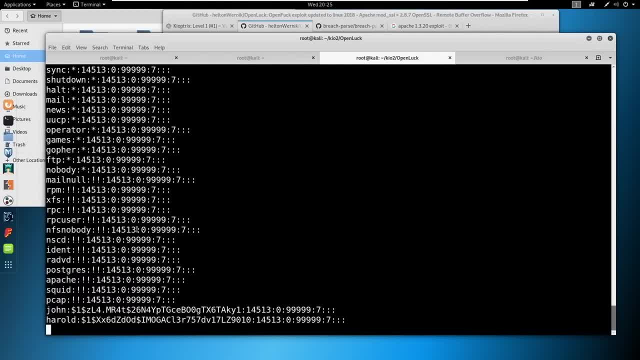 File And we would combine those. We do something called unshadow, which basically combines both the files and would allow us to at least go into hash cat or John or whatever and try to crack those. I've got a video on cracking that. 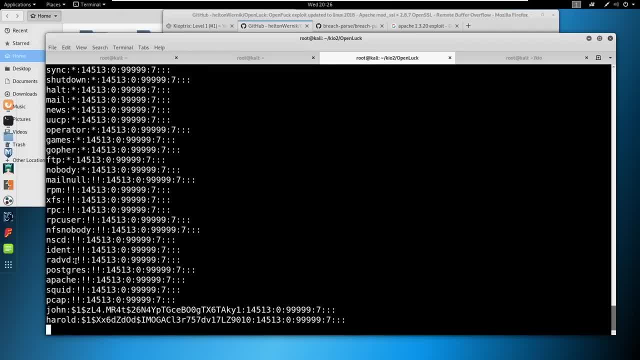 We will cover this again at a later time, but if you want to cover it sooner than later- you don't know about this topic- You can go watch the video- I have my YouTube on cracking hash cat, or Linux hashes with hash cat. 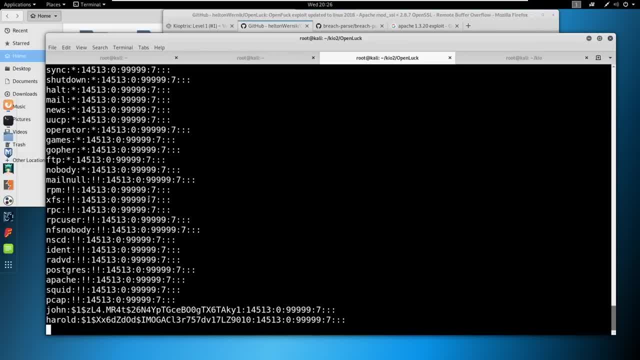 So it's pretty straightforward. but this is one of the most important things to dump Now, when we're using the ARP and we're using route and net stat, basically all I'm doing is looking for other network connections. It's possible that this is a dual home computer. 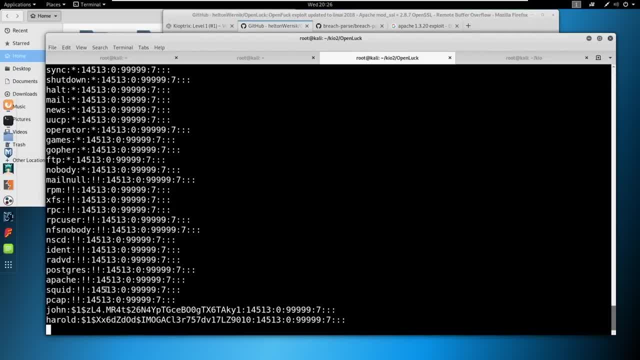 It's running two NICs. One of the NICs is on one network, One of the NICs is on another network and you're able to talk to a whole new subnet of networks. So it's important to look at where your routing table lies. 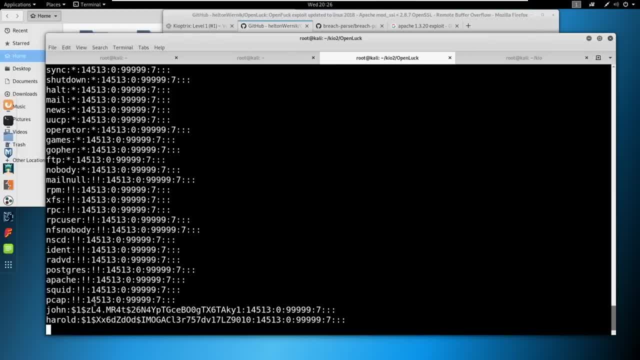 what connections you have with net stat and ARP And yeah, So anyway, I'm not going to spend too much time on that. I do want to go into Metasploit really quick and show you some things with payloads and then we'll go from there. 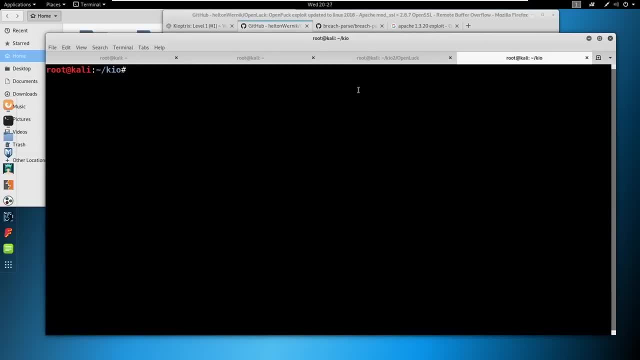 So let's just go into a new, new tab here We'll just say MSF console. All right, So let's repeat a step from last week. So what we did was we found the SMB, and let's try that again. I'm just going to type search SMB. 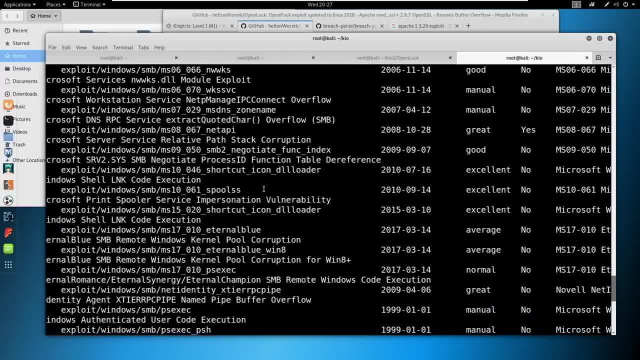 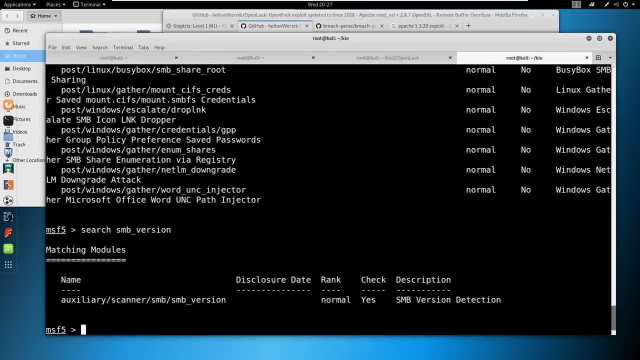 and it's going to bring back a lot of stuff. Remember, we're looking for SMB version and we could just type that in. That would actually make it easier. Okay, So let's just copy this. Remember again, there's the different types. 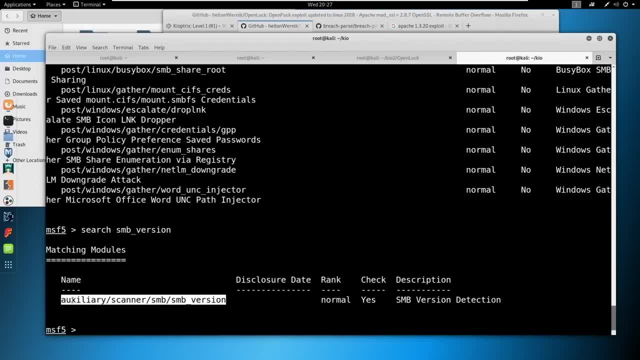 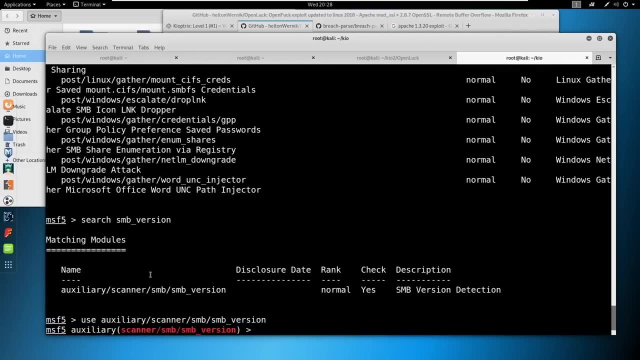 There's the auxiliary exploit, post-exploit. So we've been doing auxiliary this entire time. Now we're going to start going into exploitation in terms of modules. So first we'll use this, We'll paste it And what I like to do 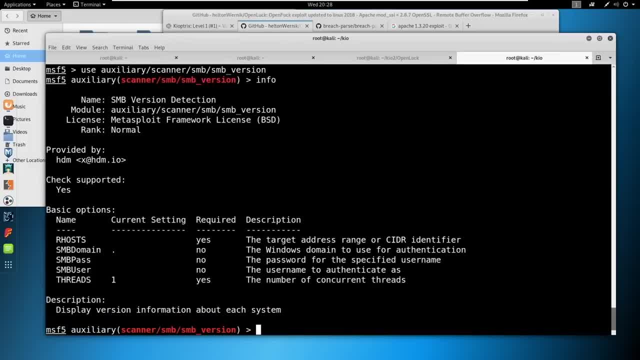 I like to come in here and I just like to type info. It gives you a little bit about it. It tells you the basic options. You know. it's just an SMB version detection. It's more important when it comes to exploits to know exactly what you're running. 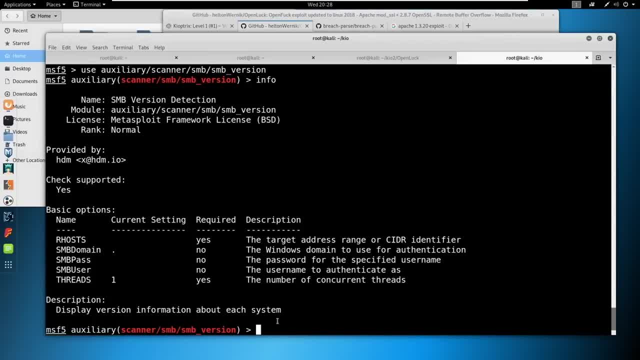 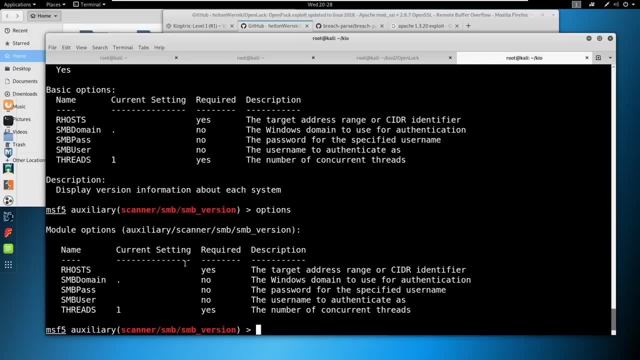 and sometimes to give you a little bit more information on the module itself. So we need an R host. Also, you could just get the basics again from just typing options and not have all that information. So R host, That's the remote host. 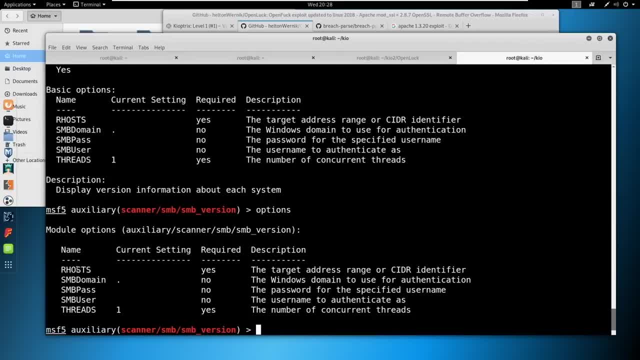 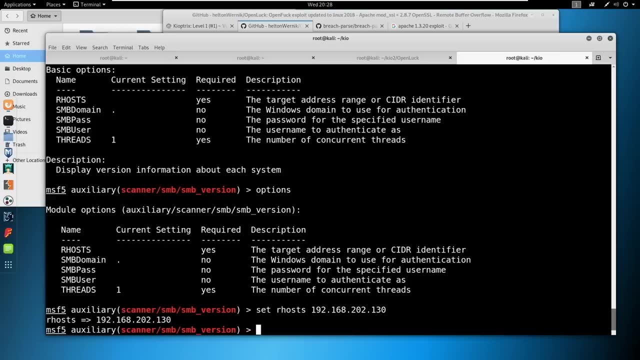 That's what we're going to try to exploit, or talk to, at least So for me. we're going to set the R host 192.168.202.130.. And we don't have an SMB pass or SMB user that we need. 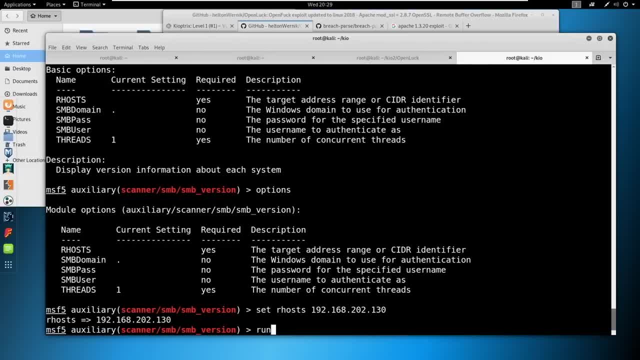 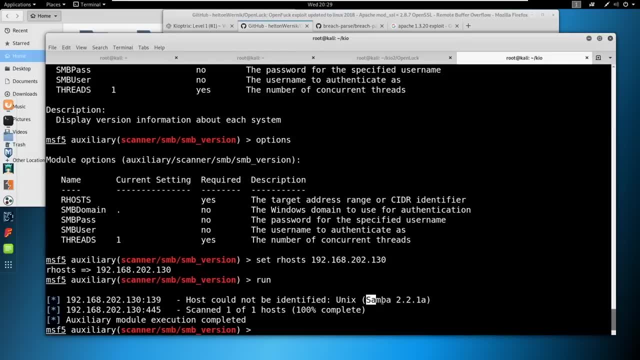 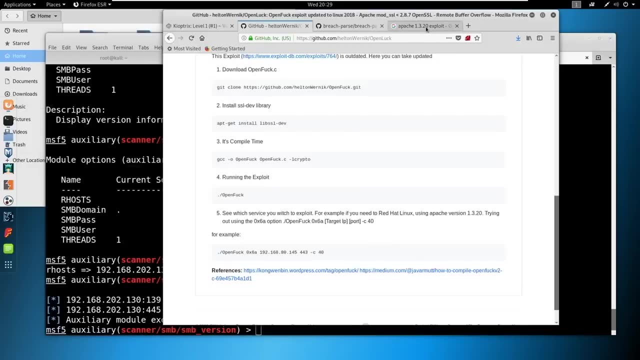 because remember from last time this was just giving up information on a default login. We run it. We see that there is a Samba 2.2.1a type here for SMB right, So we're going to go and go to Firefox. 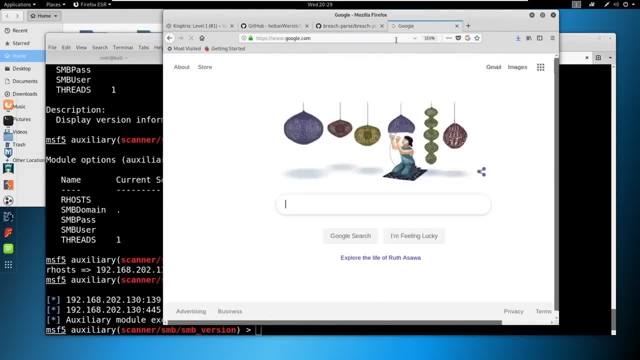 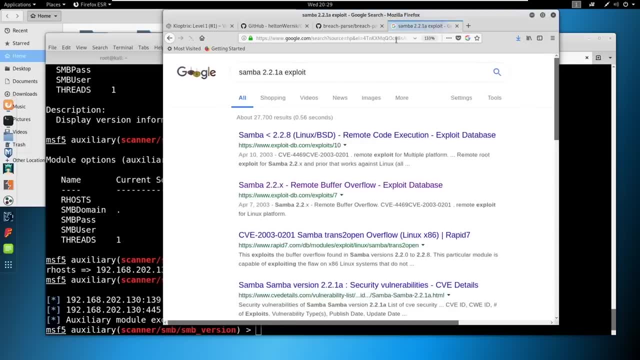 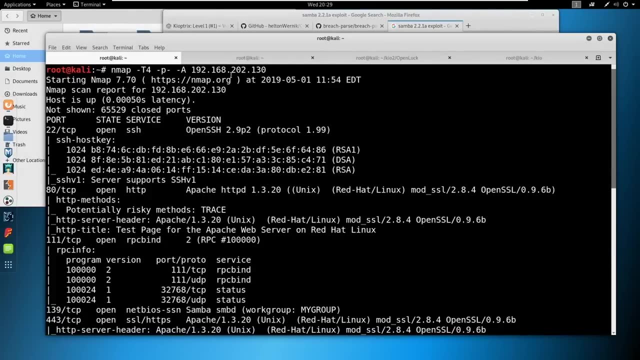 Again, we're going to say Google And we'll just paste that say exploit, And we did have a version in here, I believe. Well, we already know, right, We know it's Red Hat. I'm wondering if the version came out in the SMB. 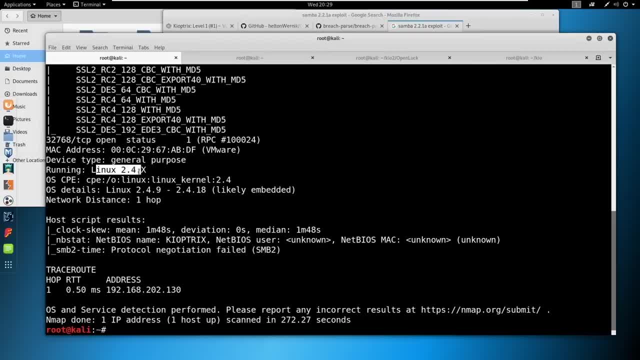 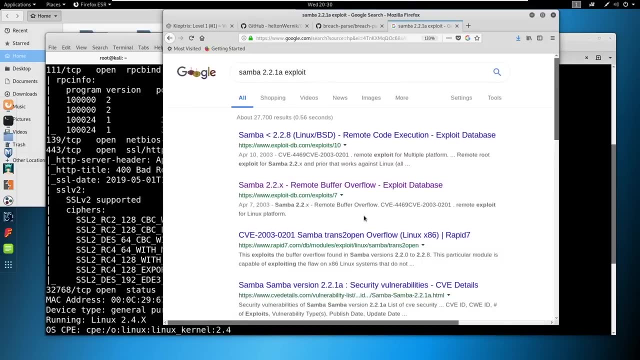 Sometimes it does Just Linux 2.4.. Let's see, Let's see. No, nothing came out there, Okay, But we do know it's Red Hat. So there's a couple different ones in here And you see, the name of it is actually under this trans to open. 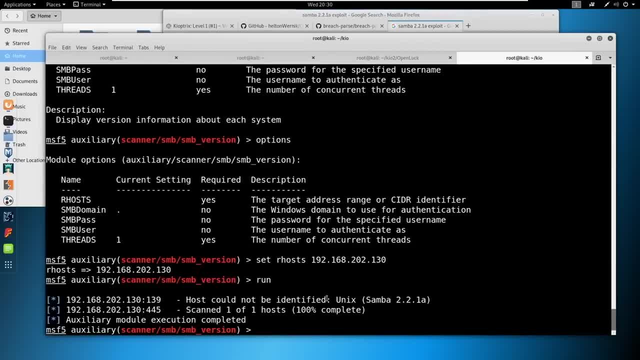 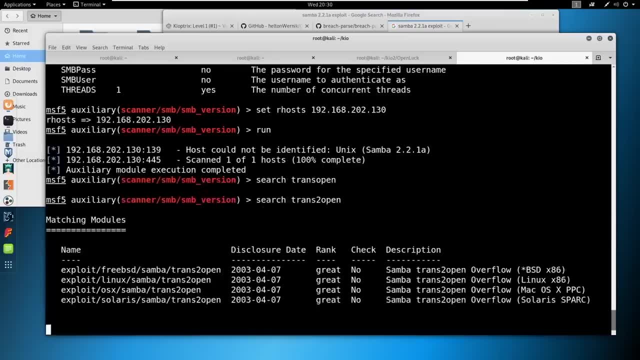 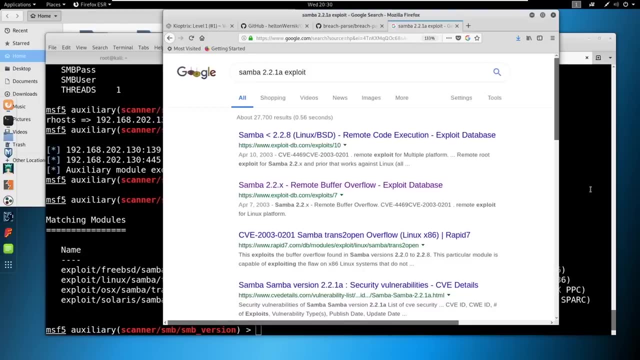 So what we can do is we can come and we can say: just search that trans to open, But if I put the two in there, that would help. Okay, And the reason we're seeing so many different ones in this Google search page is because likely. 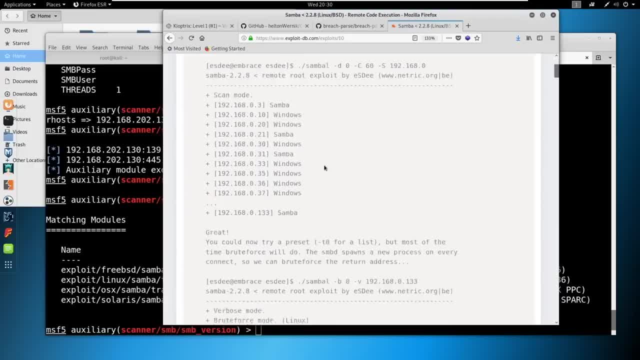 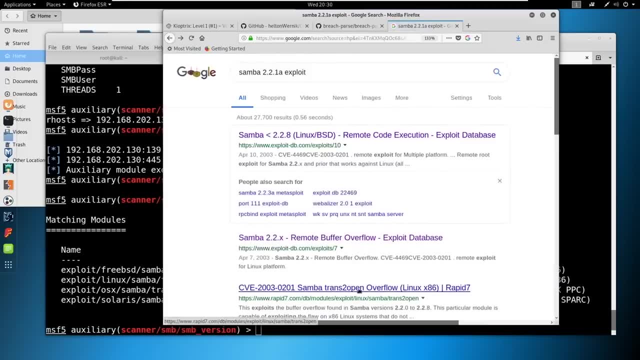 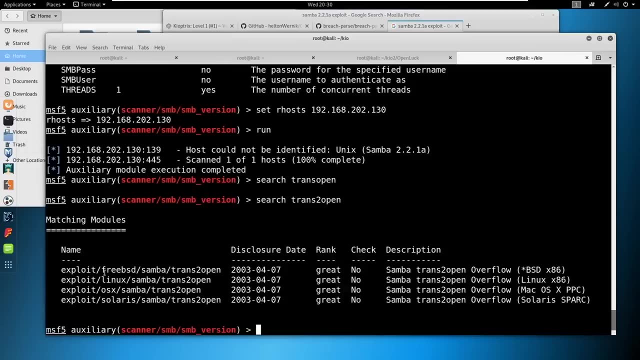 let's see what they've got. Likely, these are custom written exploits from exploit DB And they also have some- you see, the rapid seven that ties into Metasploit. So they've got Metasploit module information. So you're going to see quite a few. 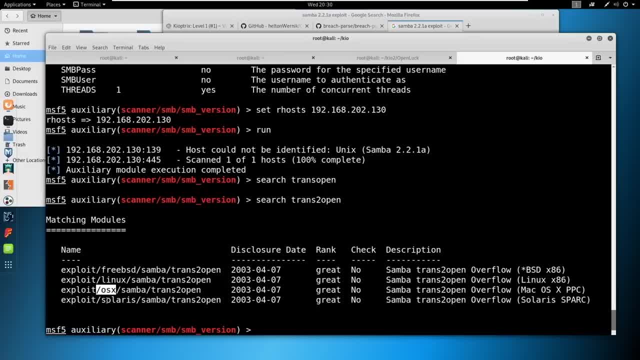 And also on top of that there's one, two, three, four separate modules for the different types of operating system. So we know we are running Linux, So I'm just going to go ahead and copy this. We're going to say: use paste. 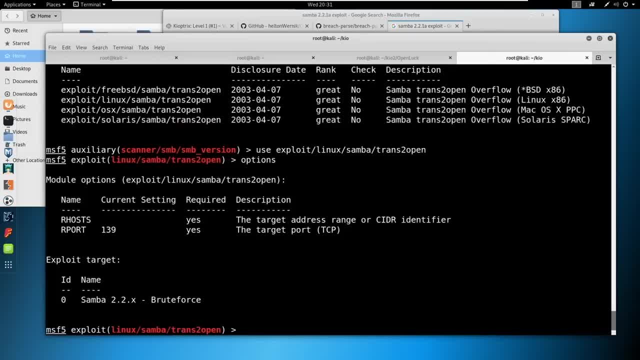 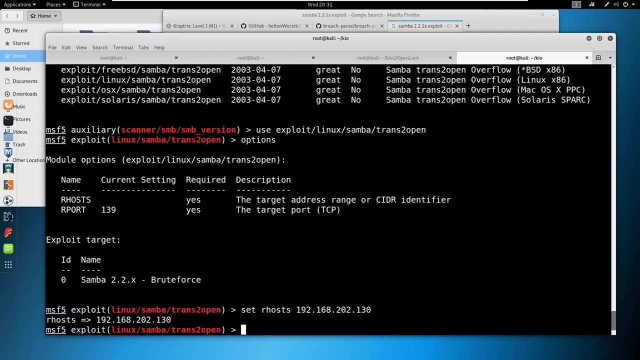 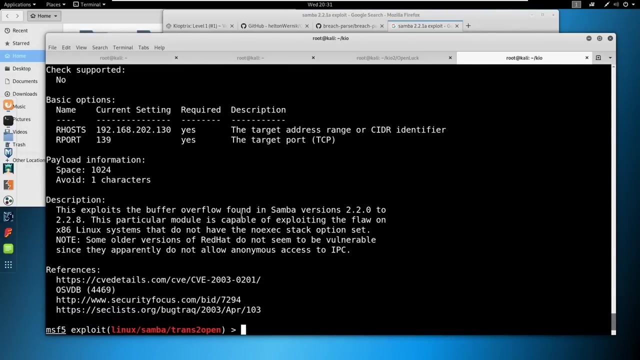 Options And again we're going to set the R host Also. again, good to read info before we fire off. So this exploits the buffer overflow found in Samba versions 2.20 to 2.28.. Okay, This particular module is capable of exploiting the flaw. 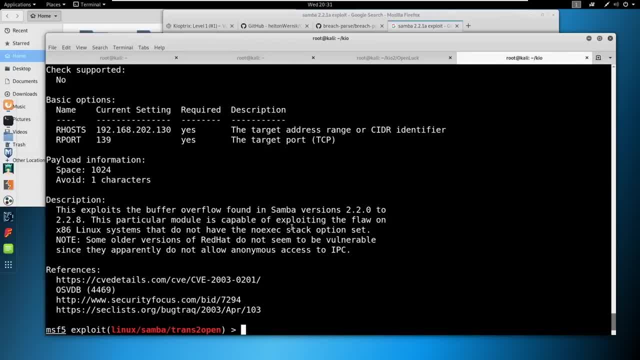 and x86 Linux systems do not have the no exec stack options set. So we are meeting these conditions in terms of version x86.. And it's talking about Red Hat older versions. We've confirmed we're on 7.2. So I don't know, in terms of older, what that means. 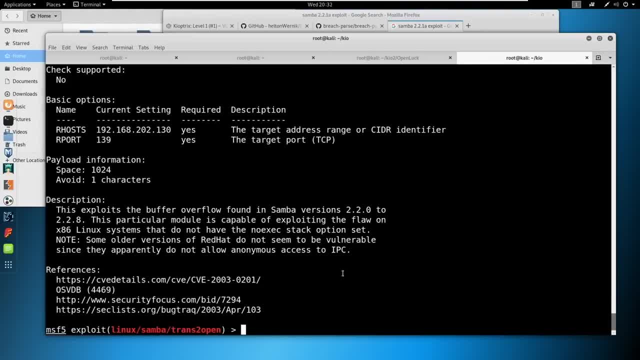 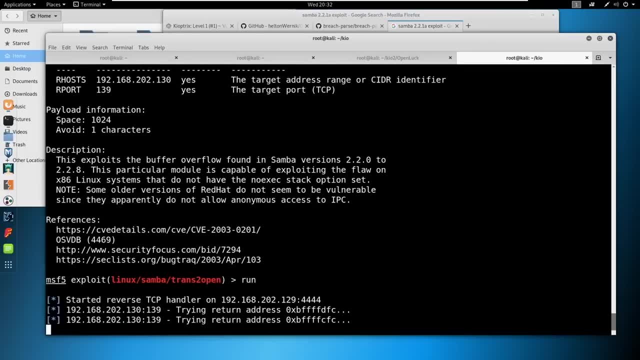 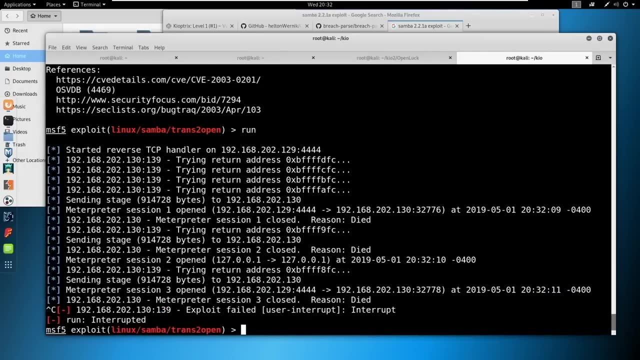 but I would be comfortable enough trying to fire this. So if we say run, Or you could type exploit because it feels cool, All right, Control C, that You should be having the same issue. So what's happening is you're getting a session open. 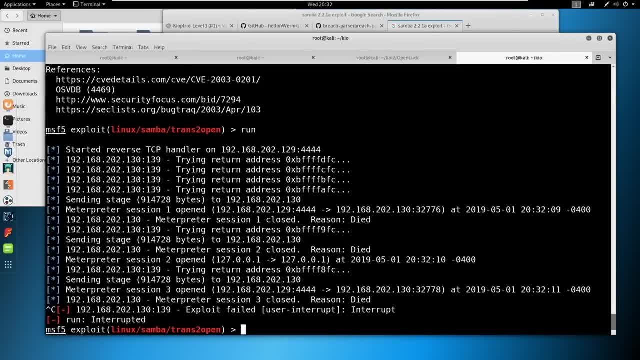 That means you are actually talking to the computer, You're exploiting it. Something is working in your favor, And then the session dies immediately, which means something's also not working in your favor. My antennas go off right away to something to do with the payload here. 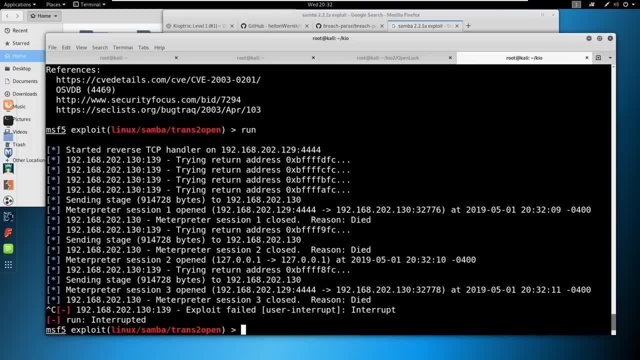 And when I mentioned earlier that that was going to be payload related, well, here's where it comes up. So if we go into here and we type in options again now, you could see something that was not here before. It gives us the payload options. 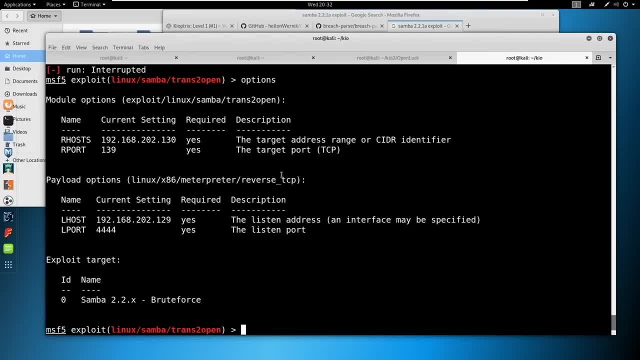 It says: okay, will you cancel that? So maybe something is wrong And what we can do is we say: oh okay, I'm running Linux x86 from interpreter reverse TCP. We can try to change this into a bind TCP. 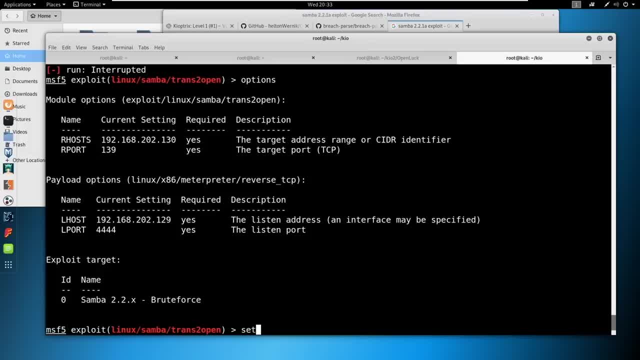 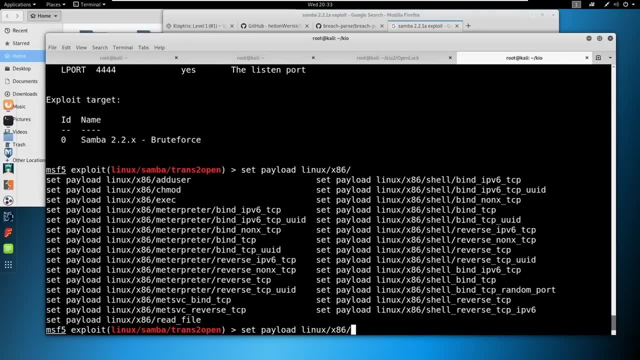 And there's so many payloads, Like we could say set payload, And we come in here and we say Linux, And we know it's x86 because that's what's available for this, We double tap: Okay, so there's a bunch of stuff in here. 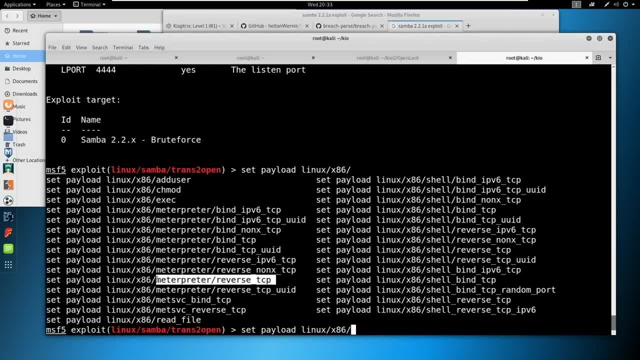 Now you saw we were using interpreter reverse TCP. There is a shell bind or there is a meterpreter bind TCP- right, But we can try to do this if we're dead set on getting a meterpreter shell But uh, but when we try this, 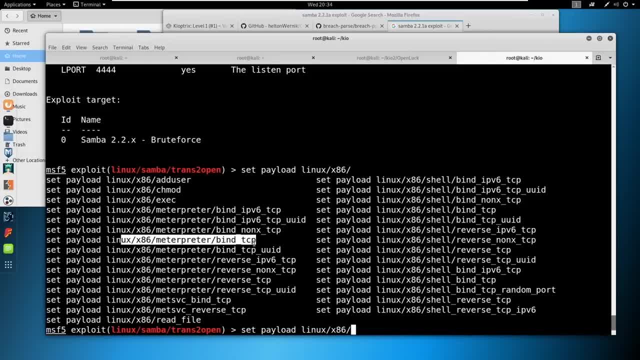 it's not going to work. I'm just saving us a little bit of time here, So this one won't work. We can come through here as well And we can look at some of the non-staged payloads, Remember. do you see the difference? here again. 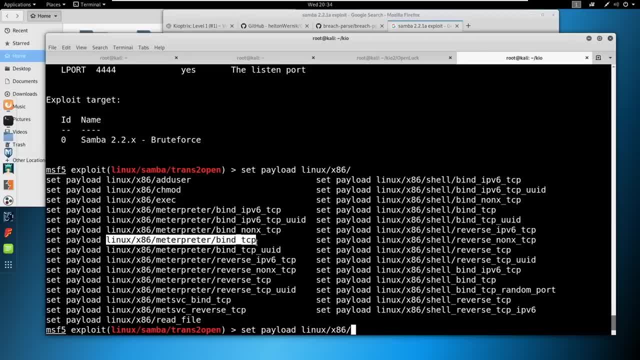 when this is coming up. You see the forward slashes. We're talking staged. You see no forward slashes after the shell. here You're seeing a non-staged payload. So, because our staged payloads are not working, we're going to try a non-staged payload instead. 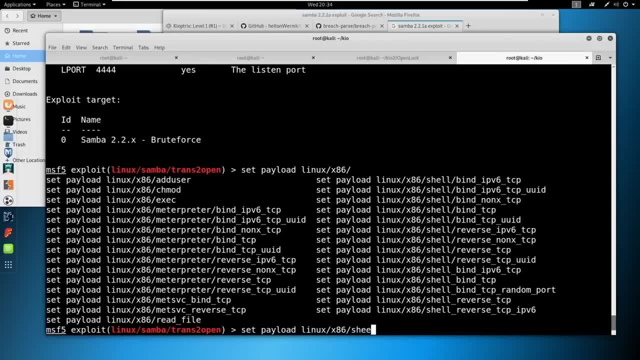 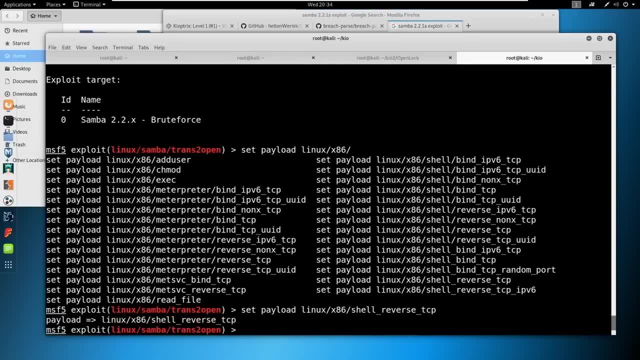 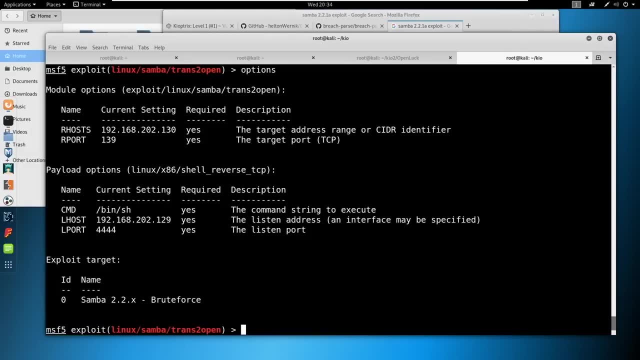 So we can try a Linux one and see if it works. So we'll just say: shell, reverse TCP Options. okay, Sometimes they come into options because what happens is when you set a new payload it actually erases everything that's set under the payload before. 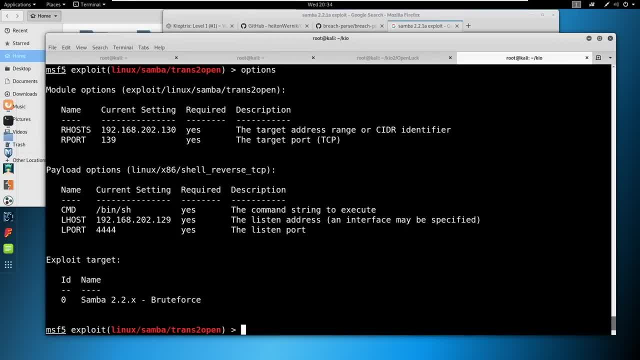 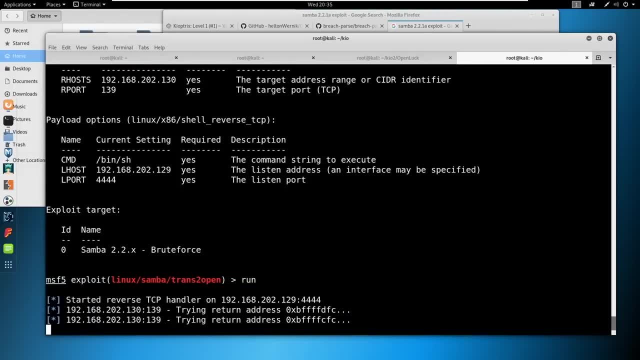 So it just tells us the command it's going to run, the L host, the L port. It all looks fine. Sometimes it erases though Type in run. Let's see if this works. I honestly haven't tried it with this one. 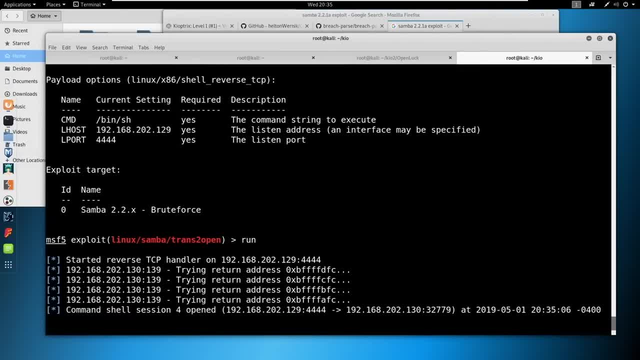 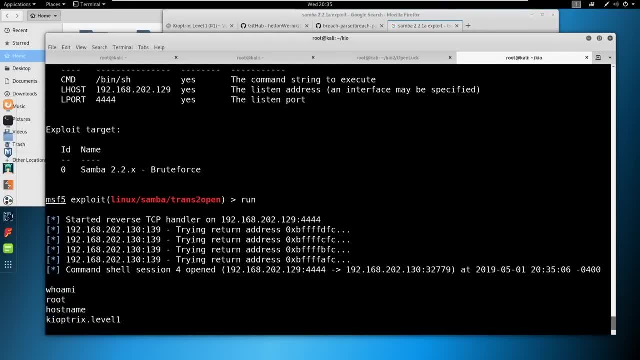 This one works, So I'll show you the one that I've tried it with before after this. Okay, so we can say who am I And we can say host name. So again we're root And again we've exploited. 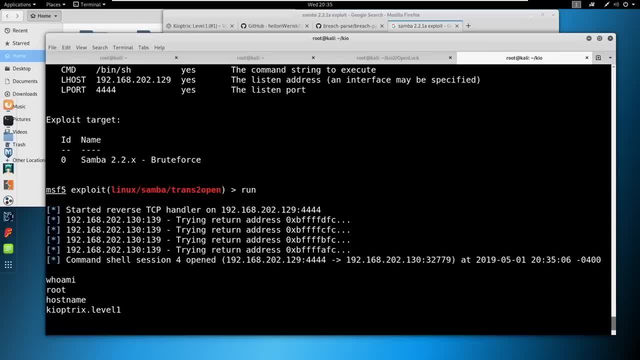 So this is pretty cool. We got a shell here. There are some cool things that we can do with more advanced shells and interpreter shells, which we're going to get into, you know, next week, possibly the week after, depending on how long it takes us to do the build. 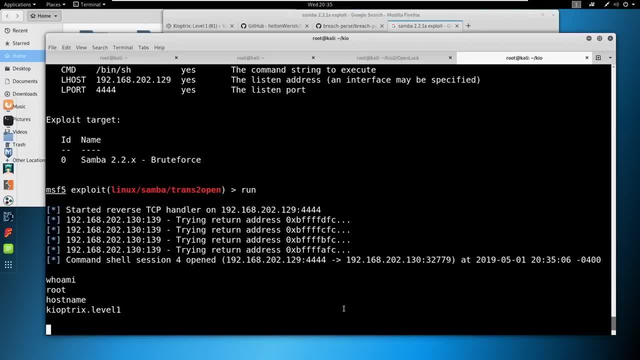 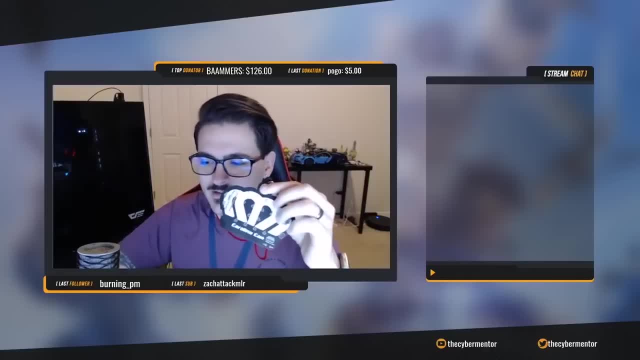 You talking about my CTF skills? Hold on, We got a guy in here talking trash. Did you not see my humble brags guys? What is this? This is Black Badge from winning the CTF buddy. Oh yeah, and all my other swag. 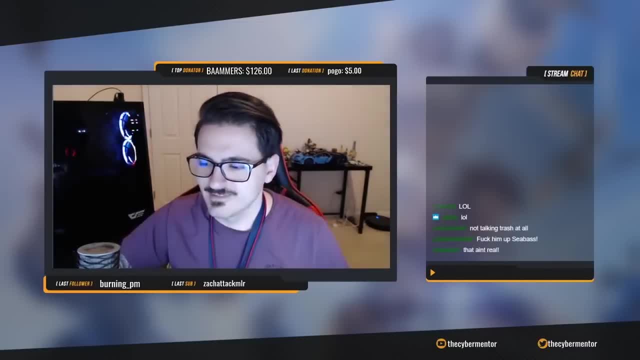 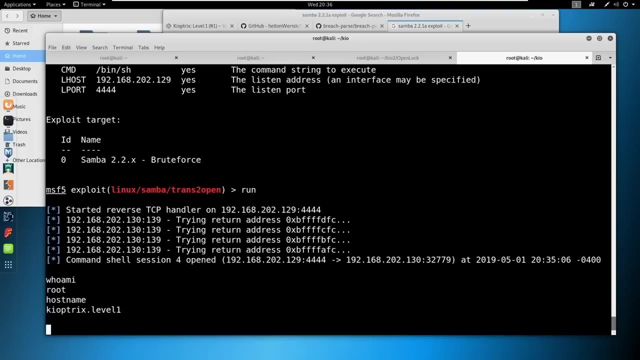 Look at this, Look at this. Don't tell me to go play some CTFs. I play CTFs. That's it. Humble guys, you've got to stay humble. You've got to stay humble, Please. 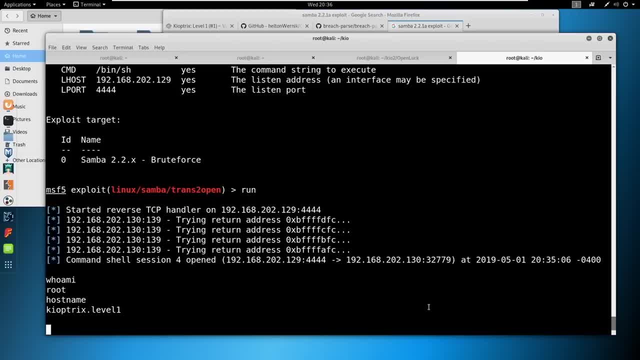 All right, So anyway. So we've got this command shell- pretty much the same thing as before. So we've exploited this machine two ways. now We've got one hell of a report to write, if we're writing a real report, right. 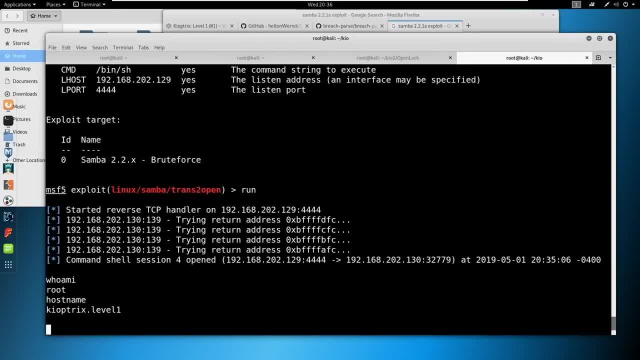 We've talked about all the other vulnerabilities that we had before. Let me see if I can pull up some of them- We don't even I didn't even capture all of them because I got tired of just writing it down- And let's see if I have. 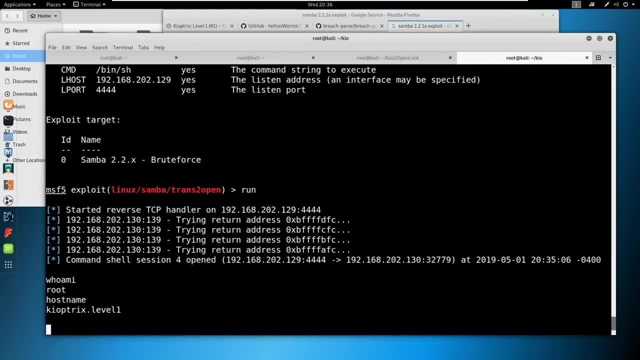 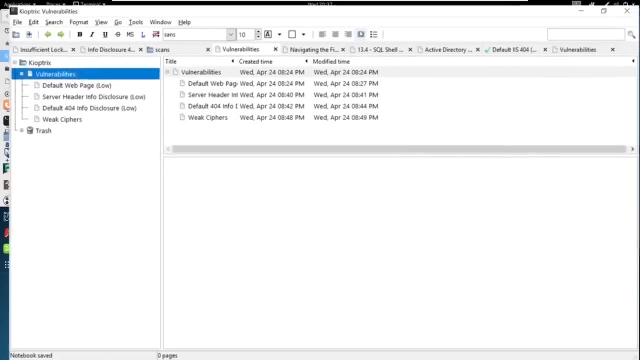 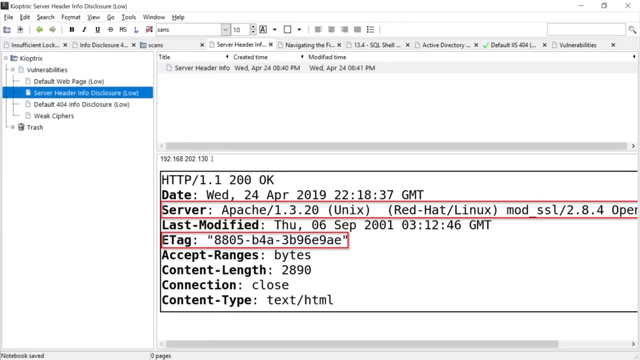 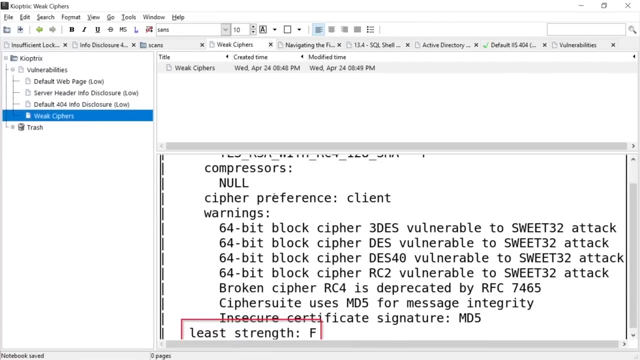 keyoptics. Can I pull this over Maybe? So remember we were going through these one by one. We found there was a default web page, There was some header disclosure, There was 404 disclosure- Weak ciphers. So we've got a lot of flaws here. 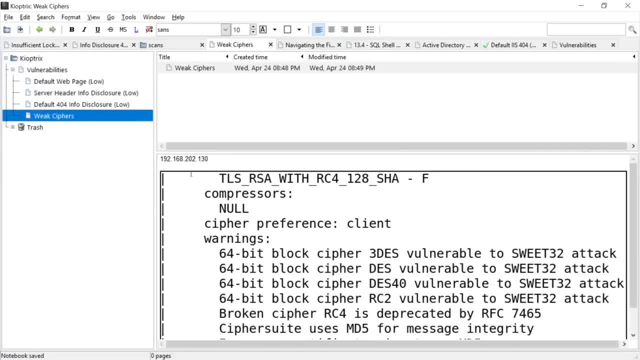 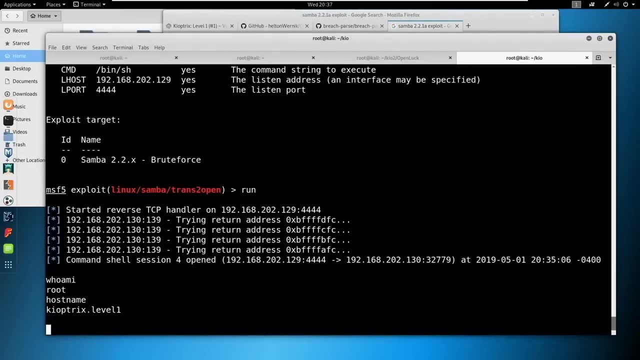 if we're going to be writing this report On top of, of course, the critical vulnerabilities that we've already found and would have to report as well. But if you're finding these vulnerabilities on an assessment, you should be alerting immediately. 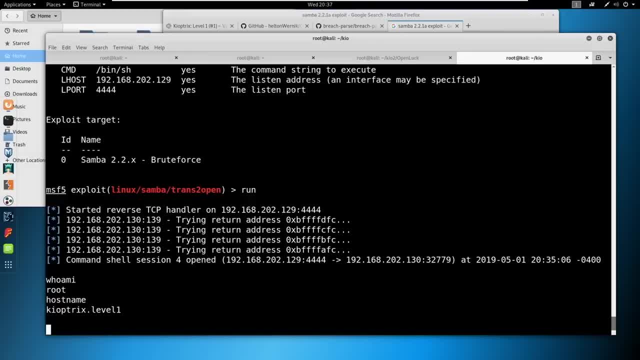 It should be an immediate stop and alert to whoever the IT manager or project manager is in charge of, in charge of things. right, For who you're you're doing a pen test for So first exploit. I would have called immediately and said: hey, I just exploited your machine. 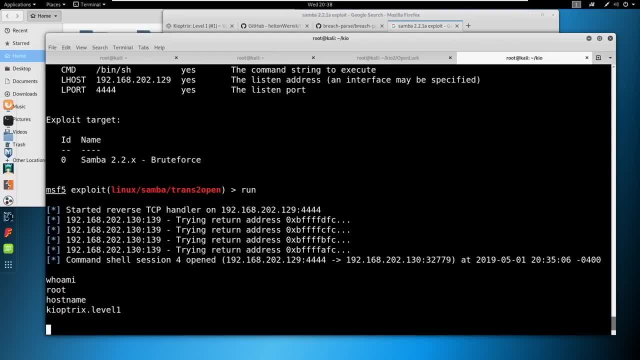 What do you want me to do? Sometimes they say, great, Go back, try again, Find all the paths you can given the timeframe. So that is it for the exploitation. I need a quick drink. All right, We're going to do one more exploit. 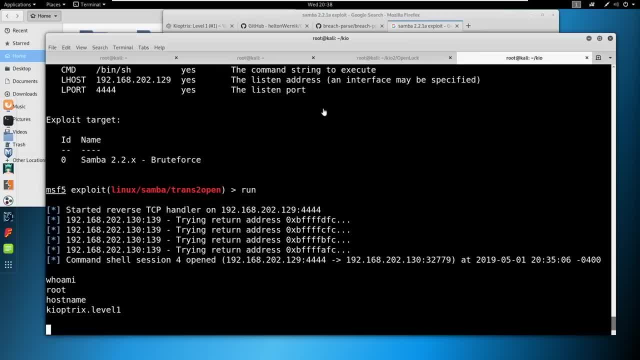 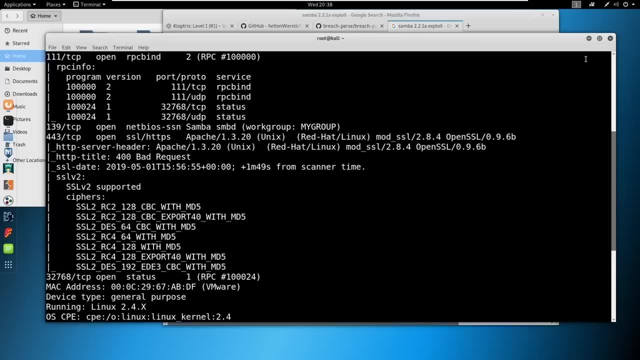 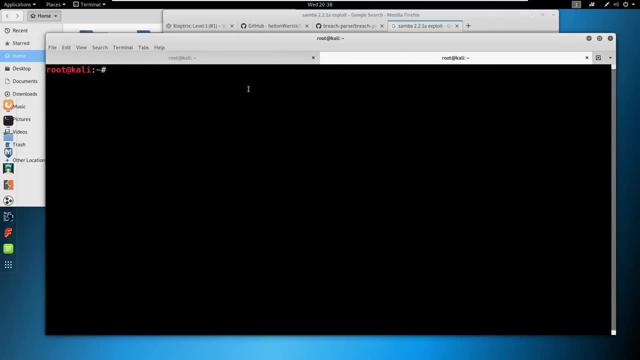 We're going to do one. We're going to do one boot to root, kind of. So let's close out of this junk here And we're going to do one together. I'm going to do something from hack the box, And what we're going to be doing is: 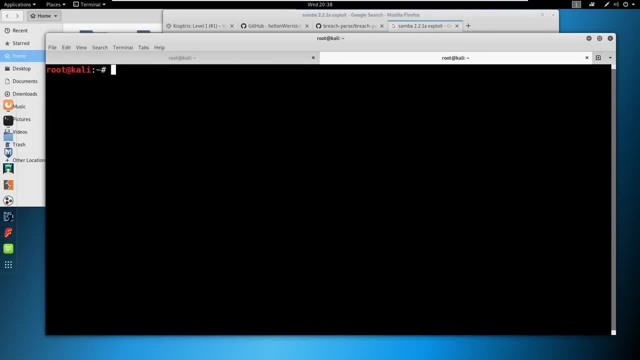 I don't even remember the name of the machine. Let me see if I can pull up the name of the machine We're going to be doing: LAME. LAME is one of the easier machines, So I'm going to get connected. 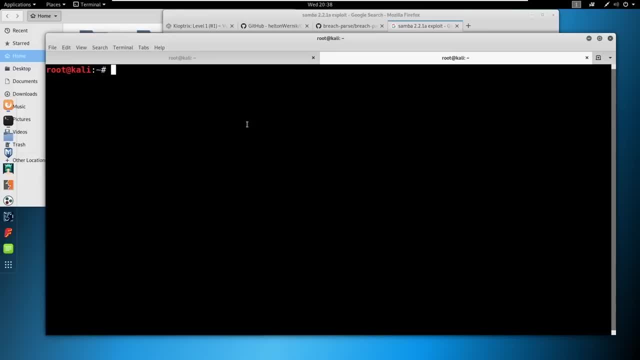 If you've got a VIP membership you can follow along. If you don't, that's okay, You can just kind of watch and soak it in. So I'm going to cd, to my downloads folder, Do my open VPN, Get connected and stuff. 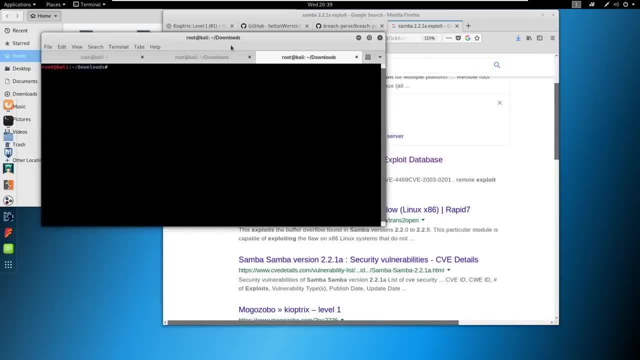 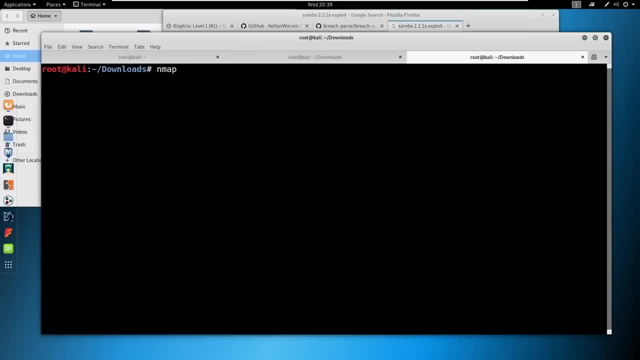 Okay, So first things first. we're going to end map this bad boy, And it is going to be sitting at 10.10.10.3, I do believe I'll let that run. I'll double check that real quick while it's running. 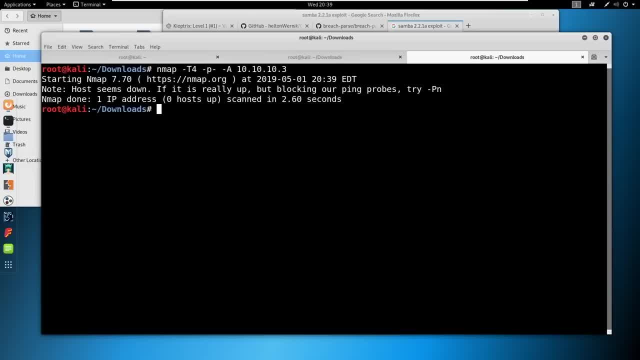 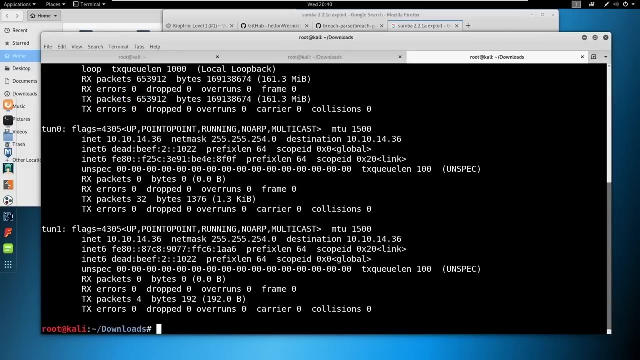 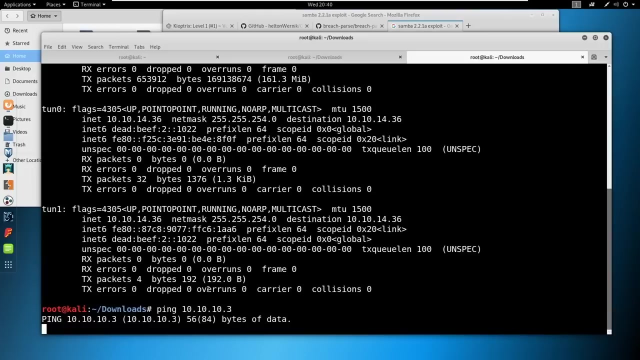 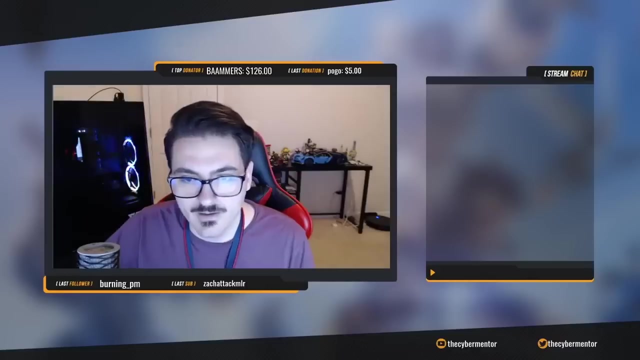 Seems down, Feels bad, Could be wrong, Should be right. Well, that's a feels bad. It's not responding, So let me go check it real quick. Until then you can see my pretty face. Okay, So I'm going to cd to my downloads folder. 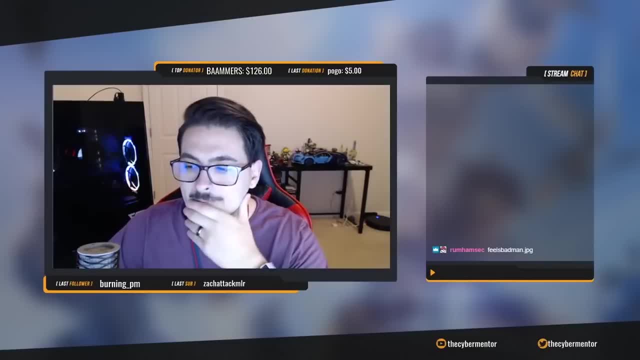 And you can do some AMA right now if you'd like to ask me some questions while we're waiting. I could be very unlucky and we could just be in the middle of a reset at the moment as well, Because it shows that it's up. 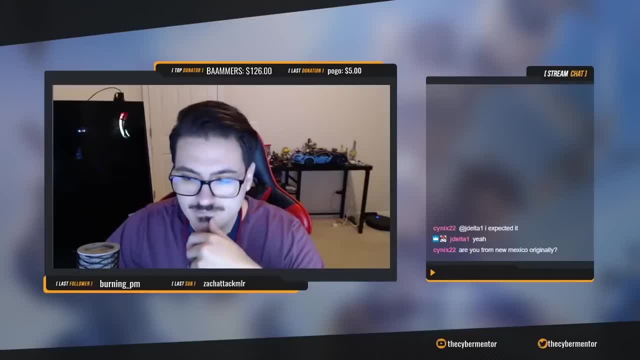 Am I from New Mexico originally? No, Okay, So I'm going to cd to my downloads folder. So I'm going to cd to my downloads folder And you can do some AMA right now if you'd like to ask me some questions while we're waiting. 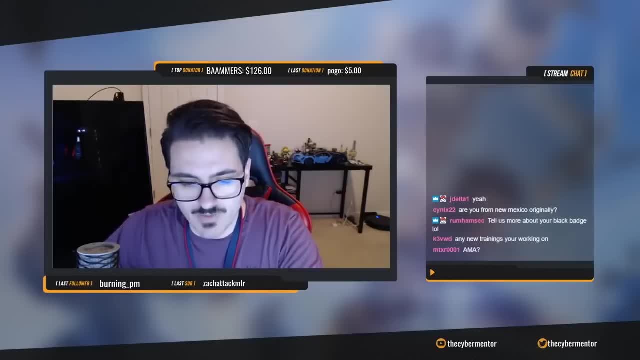 Am I from New Mexico originally? No, Have I lived in New Mexico? Yes, Okay, So it is up. I'm just going to hit reset real quick on it. Tell us more about the Black Badge. Get out of here. You've got to stay humble Rumham. 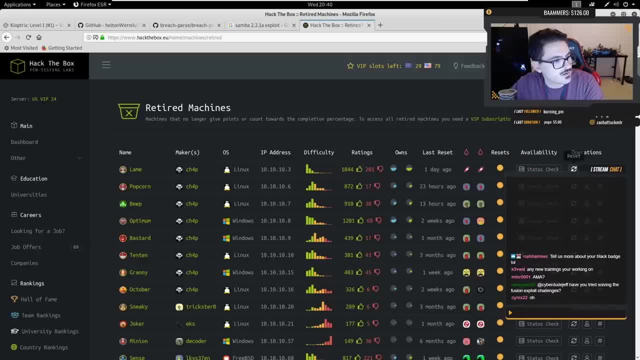 You've got to stay humble. Any new trainings I'm working on? No, Okay, So I'm going to cd, to my downloads folder, And you can do some AMA right now if you'd like to ask me some questions while we're waiting. 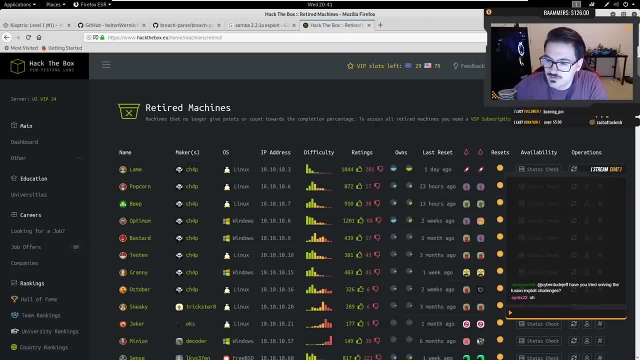 I could be very unlucky and we could be in the middle of a reset at the moment as well. Okay, So I'm going to cd to my downloads folder And you can do some AMA right now if you'd like to ask me some questions while we're waiting. 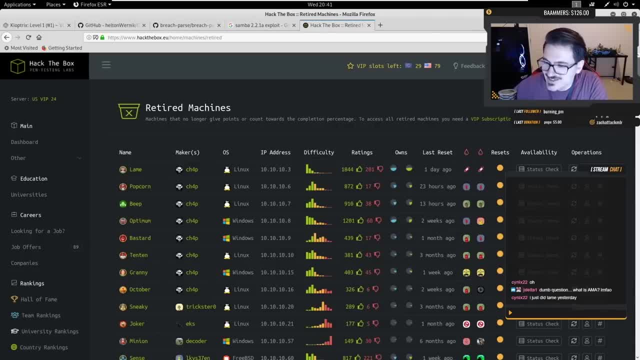 Tell us more about the Black Badge. Get out of here. You've got to stay humble, Rumham, You've got to stay humble. Any new trainings I'm working on? I've got to finish the eLearn security web penetration testing extreme by May 15th and 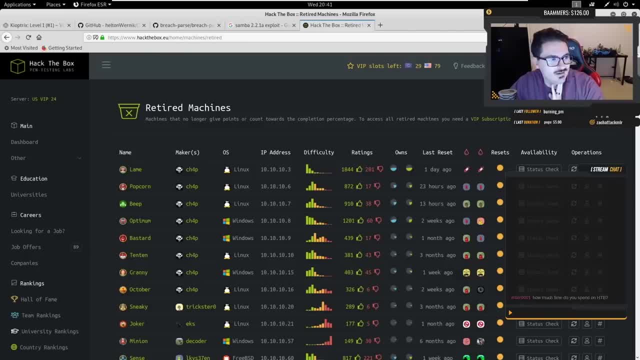 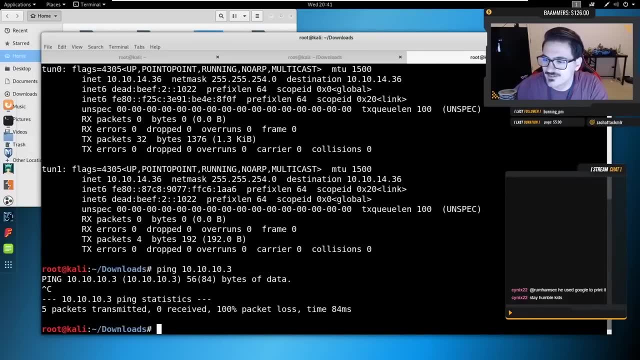 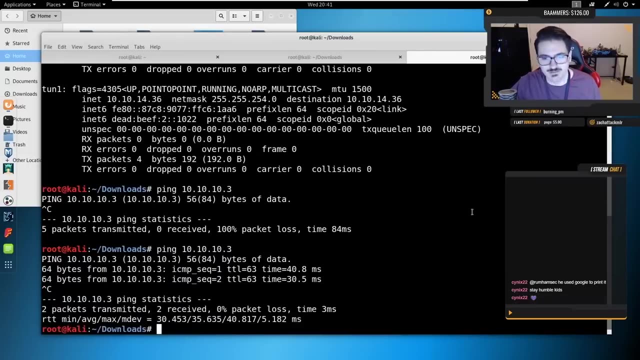 I'm like three chapters in, So I don't know if I'm going to finish that one in time. I may need an extension. Okay, Spreading fake news is a bannable offense, Gray. Okay, there's the ping. 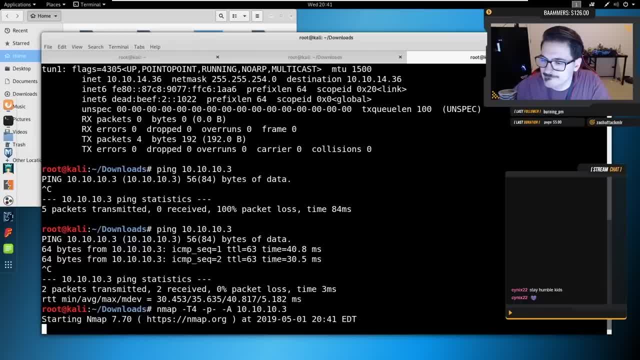 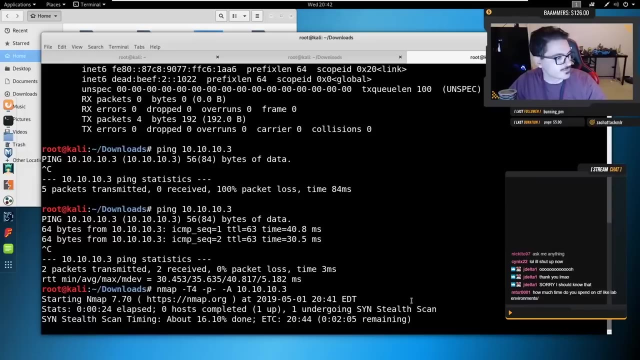 Let's end map that AMA stands for. Ask Me Anything. All right, so we're going to let this run just for a minute. It should be quick. I don't think there's a lot of ports open on this one. How much time do I spend on CTF environments? 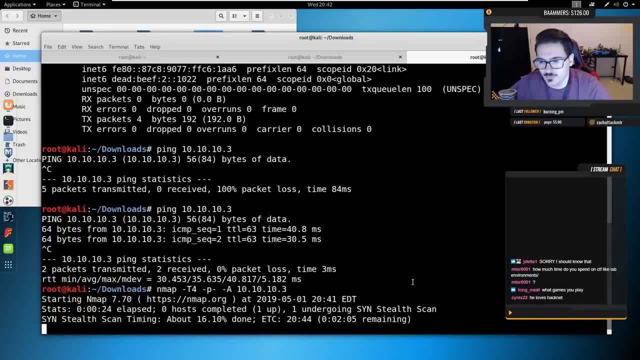 Not as much as I'd like anymore. When I get practice time nowadays I'm practicing on like Synac and doing real-world environments just to you know better my skills, because it's more realistic and you can get paid, you know. 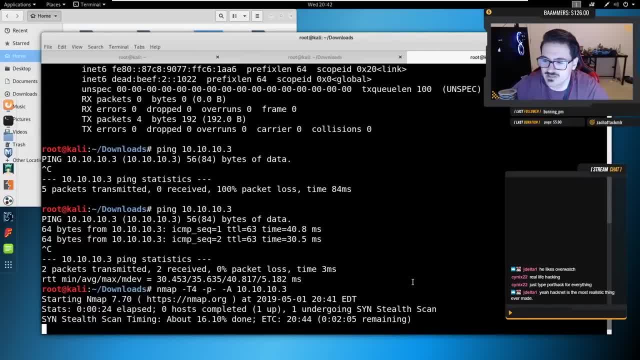 So I'd rather do that. I'd rather do that and try to earn some money- and you know better where I can- as opposed to doing the CTF stuff. The CTF Wii one was wireless, so I actually like wireless quite a bit. 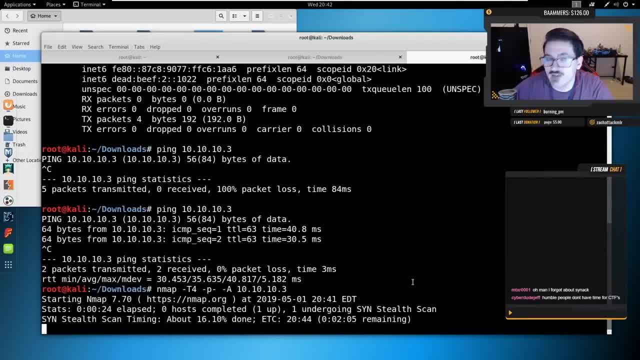 What games do I play? I do like Overwatch. We have played HackNet Does not mean I enjoyed that game. Humble, people do not have time for CTFs. Have I done Hack the Box Offshore? I have not. That is on my to-do list. 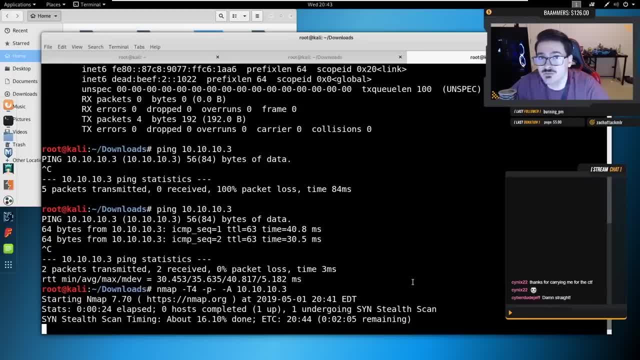 So I've got the Penetration Testing Extreme already purchased for eLearn Security. I plan on doing that together with Offshore to kind of piece them in and get some real like advanced Active Directory training in. So Oh, there was no carry Gray. 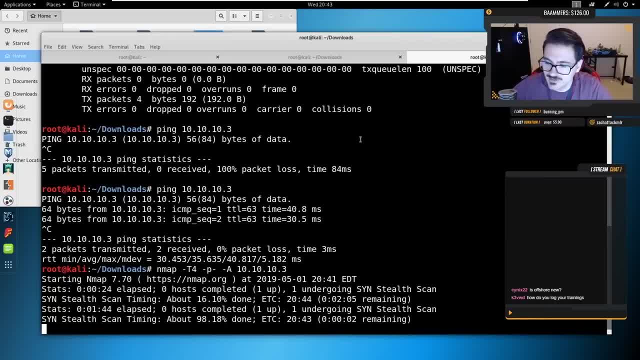 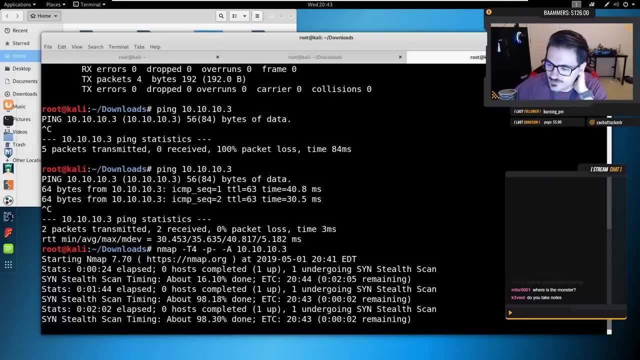 Stay humble. How do I log my trainings? What do you mean? how do I log them On a resume? We're getting there. Oh yeah, I take notes. I showed my keep notes in the beginning. Let me see if I can pull one up. 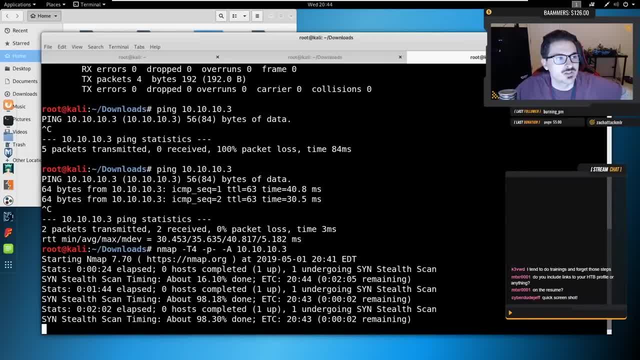 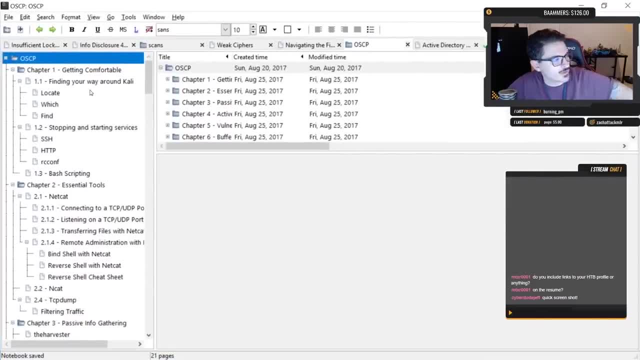 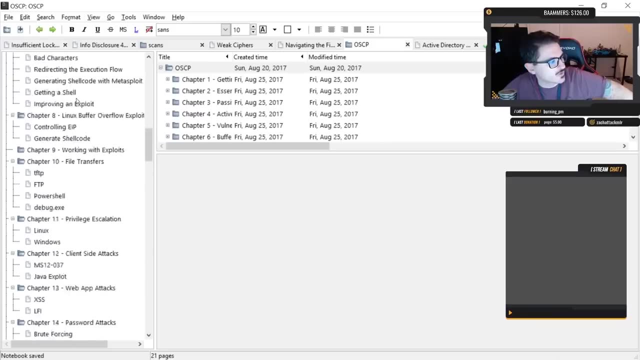 Uh, Uh, Uh. Let me make very sure that I don't disclose anything here. Like Like my OSCP, I went through every single chapter, did a subchapter and a sub-subchapter all the way through And then all the exercises. 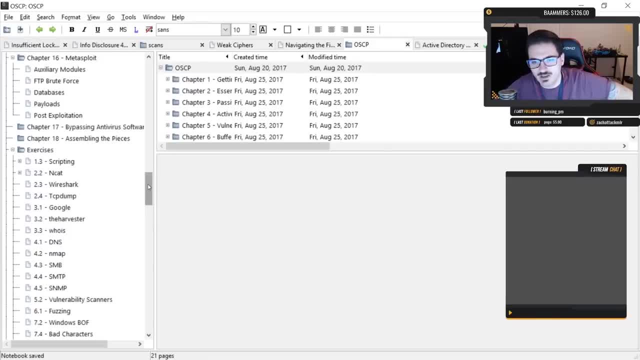 and then all the machines down below which I won't scroll down to, but you can see about how far I am down this. The more detailed notes, the better you are. Uh, This, This is keep notes. Some people like Cherry Tree. 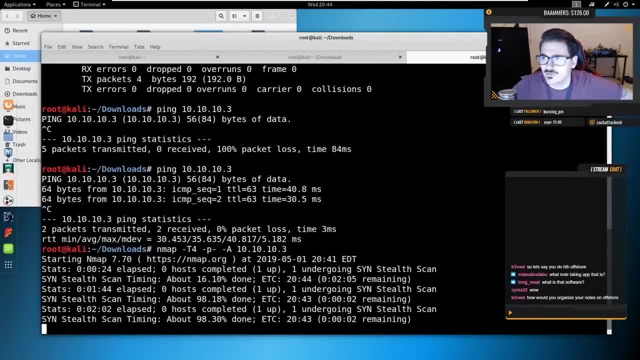 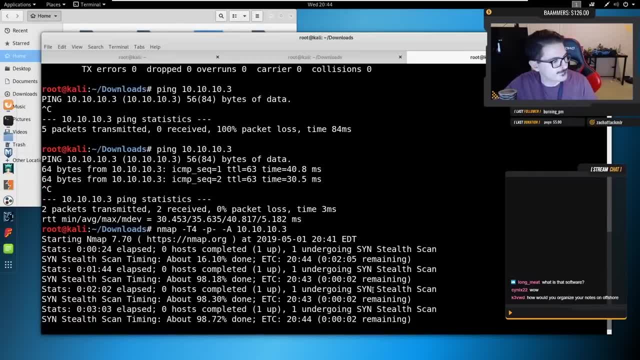 I like keep note, because keep note is more color-friendly to my eyes. I like a white background. I don't do the dark background. I know some people like the dark backgrounds. This is dragging. now How would I organize my notes on Offshore or Ross Labs? 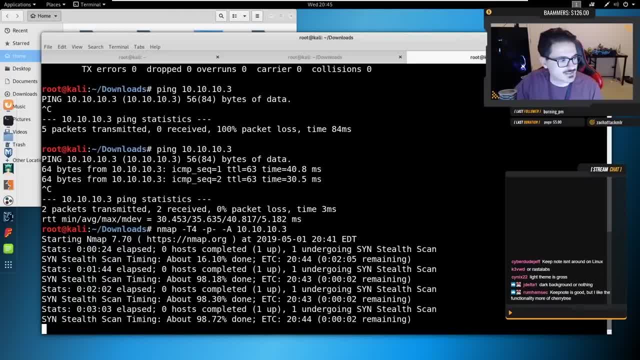 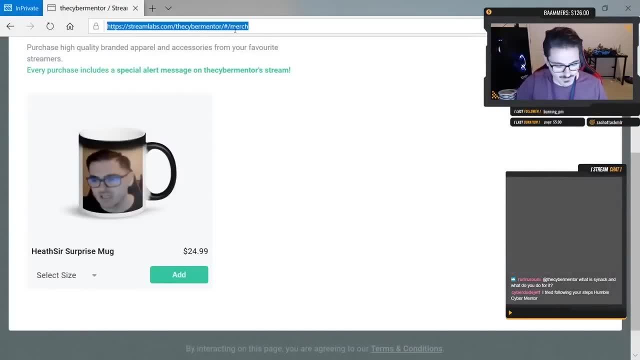 Just the way you saw it. Pretty much exactly the same way you saw it. So Cinec is a private bug bounty program. Uh, Let me see if I can bring up. Let's get my ugly mug off of the page. 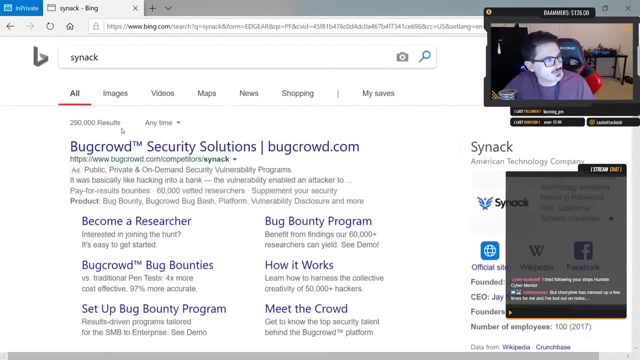 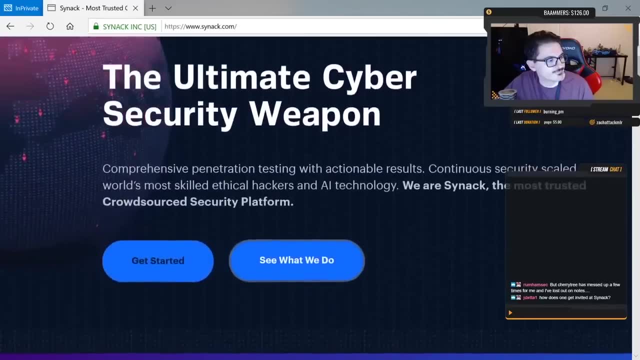 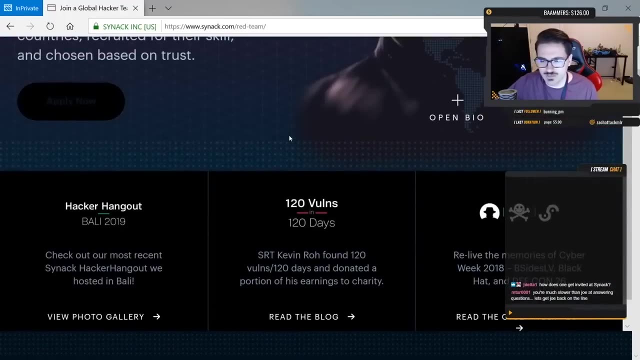 Cinec. I like how bug crowd comes up first. That's funny. So this is Cinec, Basically it is. There's the red team. You apply for the red team And you send a resume. If they like your resume, you have to do a written assessment. 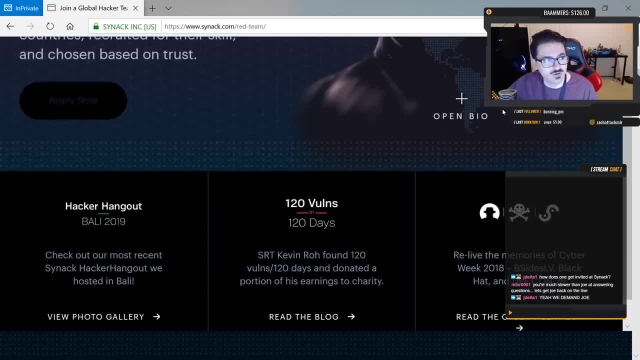 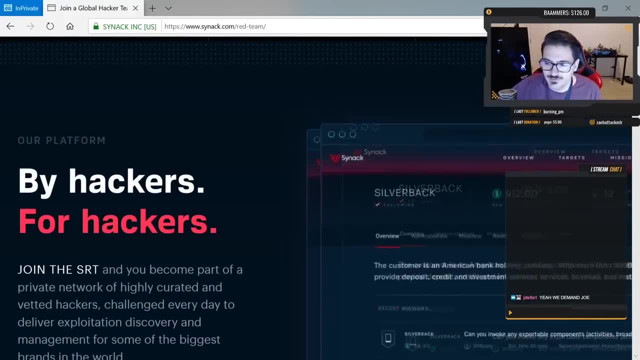 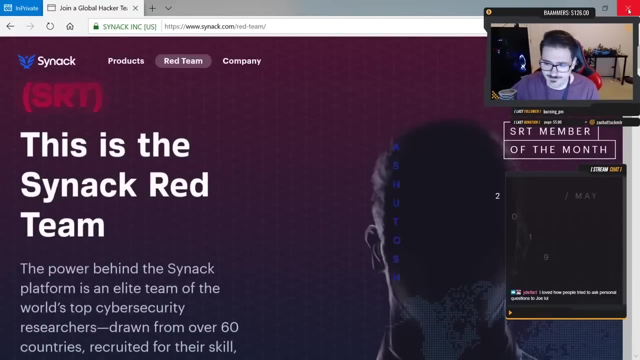 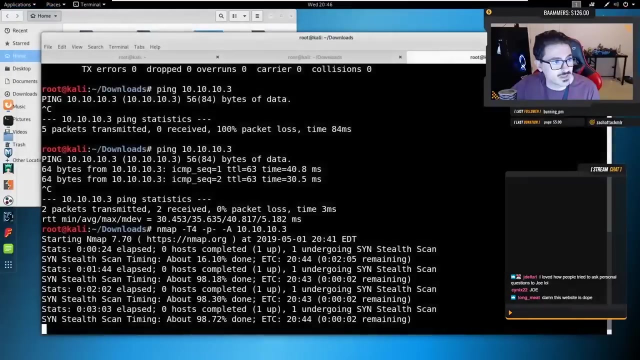 a practical assessment, an interview etc. and a background check and then you get in. So It takes a little bit but it's less crowded, so I think it's easier to earn money. Anyway, you have to do one for every type of assessment they have. 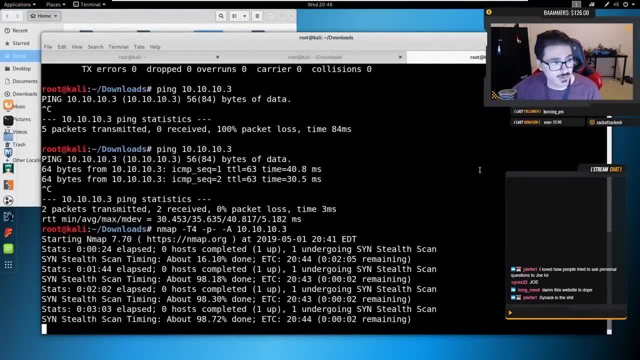 So if you want to work on web apps, you have to do web apps. If you want to work on host assessments like network, you have to do a host assessment. So there's mobile, there's hardware, there's a bunch of them. 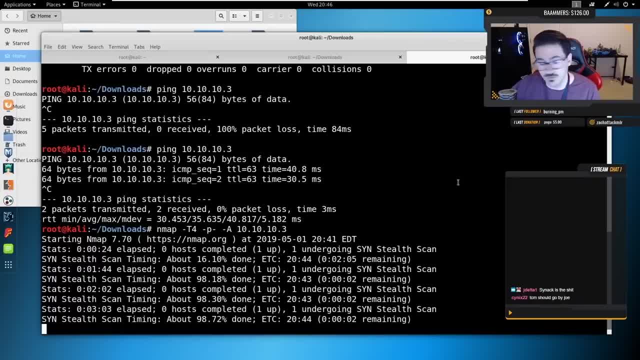 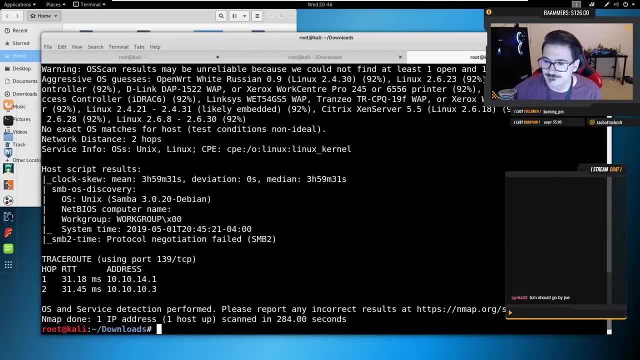 I only have host and web app done, so There's quite a few that I could still attempt and try to do. What questions did I miss? How does one get invited? You apply and try to make it pretty much. Sorry that I'm slow or MTX. 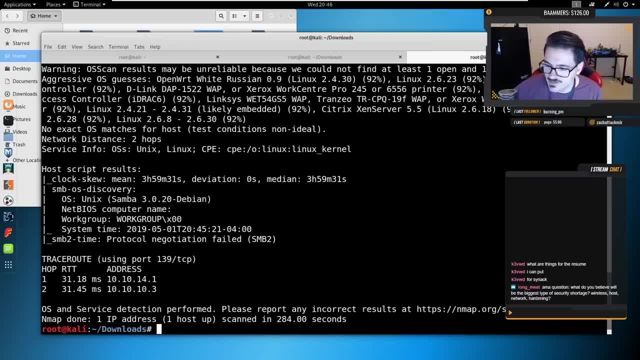 I won't answer any more of your questions tonight, buddy. I'll just ignore them. All right, We'll get back to the AMA in a little bit. So let's look at this, because we are still not in AMA territory. 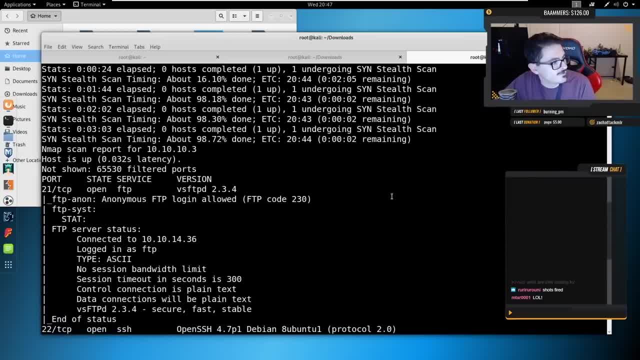 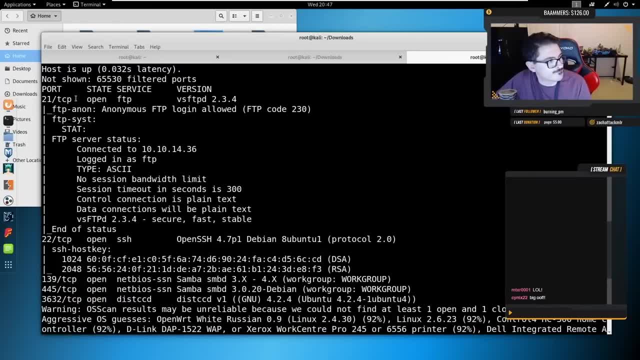 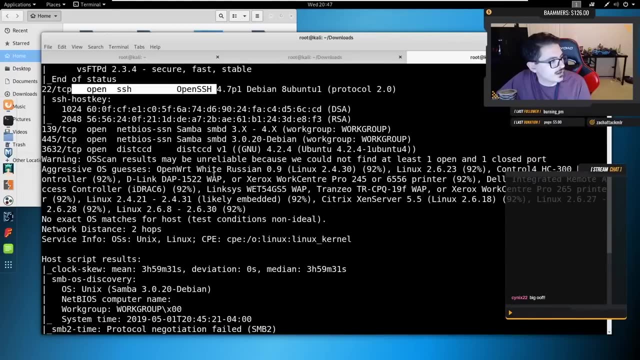 We are only at 847, my people All right. So there are a few things here. We see FTP is open, We see SSH is open And we've got SMB, SMB 139, 444.. 5, perfect. 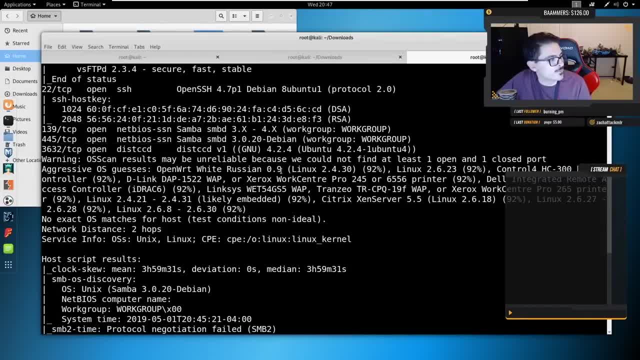 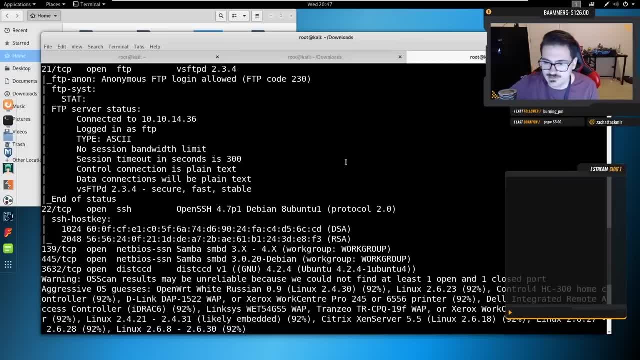 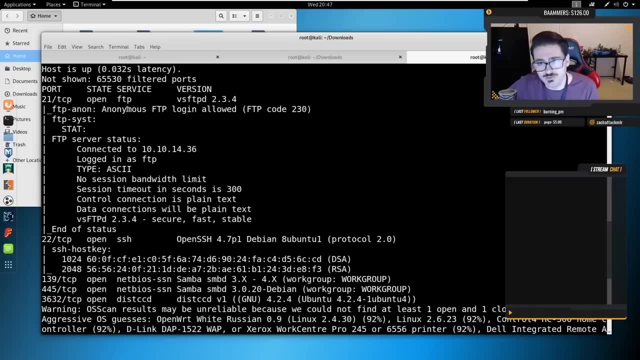 We've got 3632, which is interesting. So if we're enumerating this machine- and we're probably going to take this till 9 o'clock, so I won't enumerate everything- The first thing I would probably look at is what's running on the FTP server. 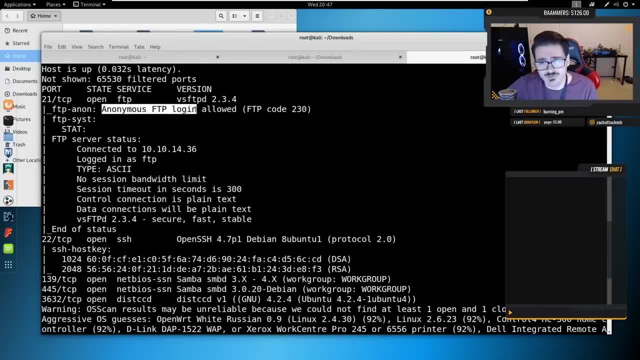 It says anonymous FTP is allowed, So what type of information could be downloaded from there Just by looking at this? Obviously, we want to look at the version We want to see. okay, is this 2.3.4 of VSFTPD vulnerable? 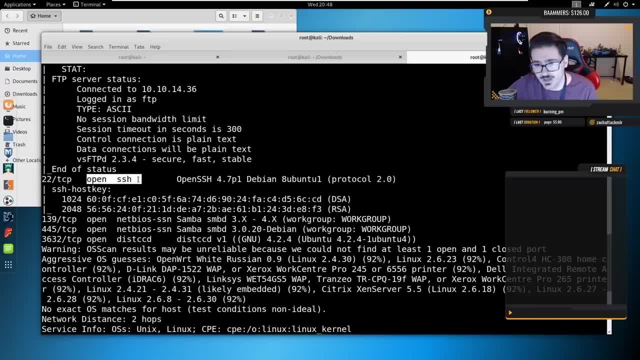 SSH. So SSH we can try to prod. Remember we talked last time when SSH is open and this is on like a pen test, not necessarily just a capture the flag When SSH is open, we're going to try to do a brute force attack during a pen test to see if the SIM catches us and if they have weak control. 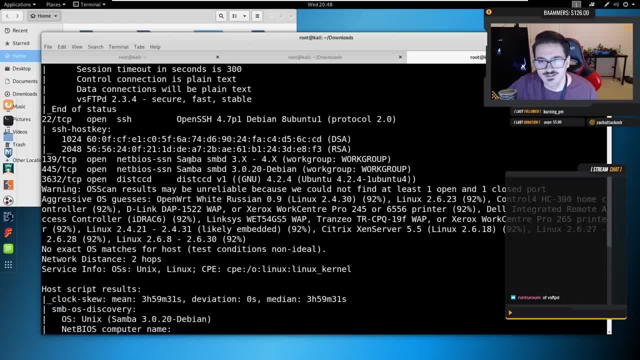 Thank you, Ruri. I know that. I appreciate that. So for 139.445, what we're doing is we're looking at these and we're saying, okay, can we connect to 139.445 and see what the version is? 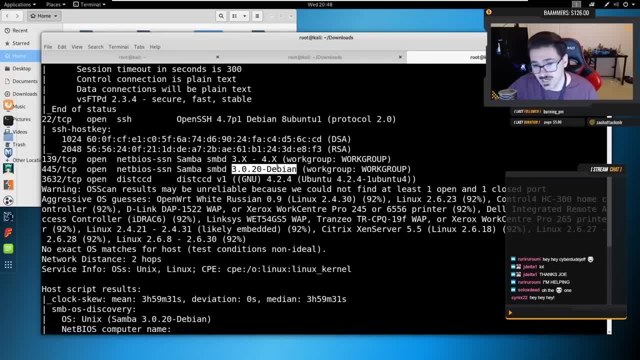 Well, we don't need the version. We got it right here already. Can we connect to it anonymously? What kind of information can we get out of the folders, et cetera? And this 3632, I've actually never seen before. 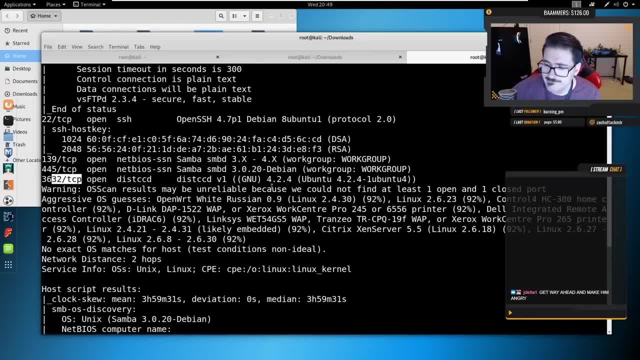 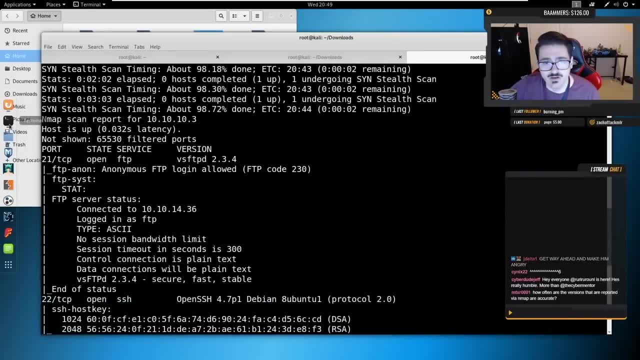 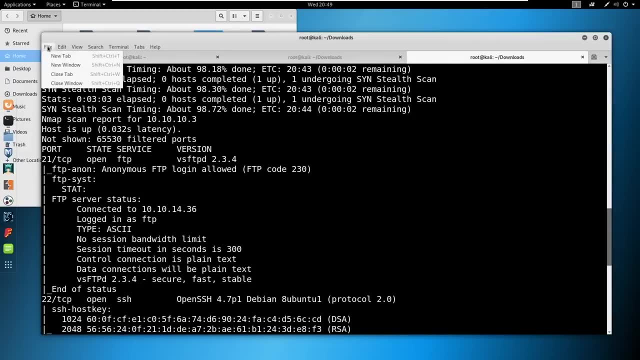 Doing this machine. So okay, So when we roll through here we can take a look at FTP if we want. So let's just open up a new tab real quick and I'll take my face off the screen. So we'll do a new tab and we'll just say FTP. 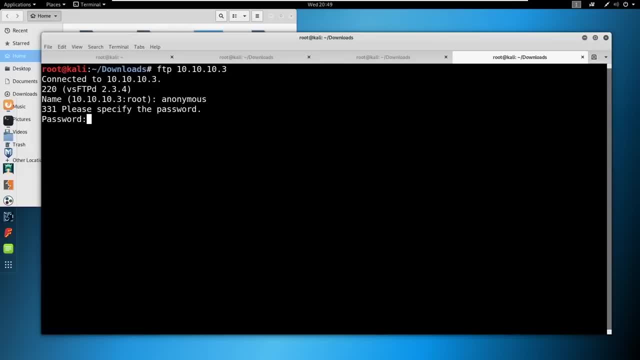 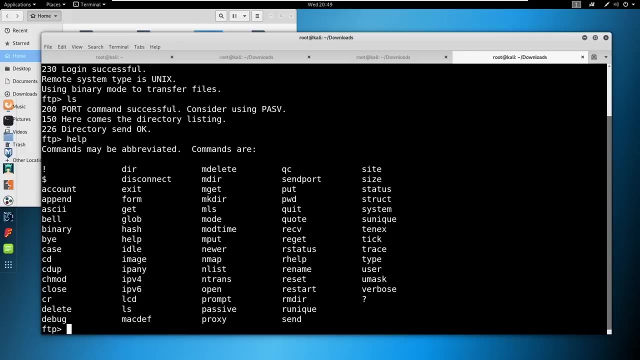 Okay, so it says anonymous logins available. So we would say anonymous, anonymous. Okay, successful, Pretty much commands. I said LS, Here comes the direct listing. Okay, Doesn't look like there's anything there, So we can put things in here if we wanted to. 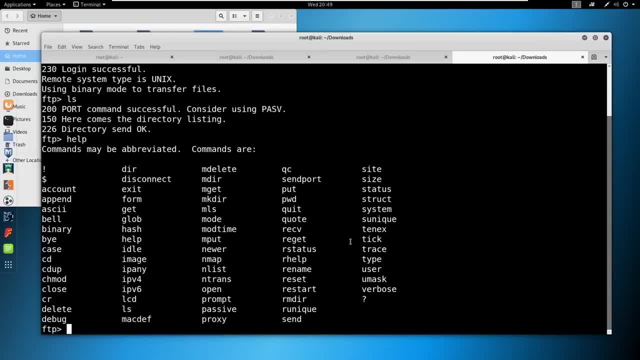 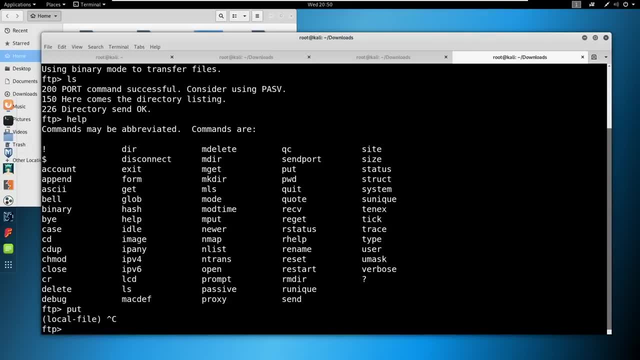 Is put available? Let's see. Yeah, we could put stuff. Let's see. However, oh, it puts right up here. However, we'd have to have a way to access this. So if we're doing like a capture the flag and this is for some reason, say, like a web server, 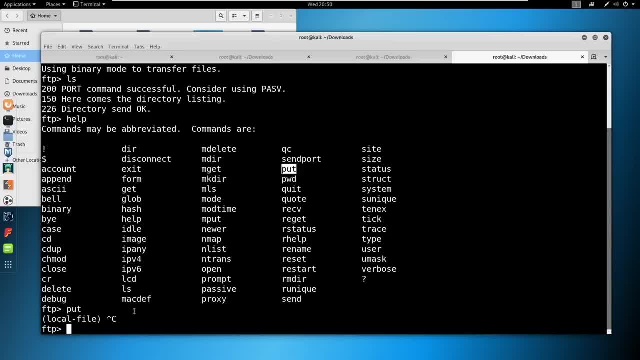 like somehow the FTP lives where the web server is and you could put something in there like a reverse shell. maybe that's interesting. Or they put some kind of file in there for you to upload Interesting Or download Interesting. But 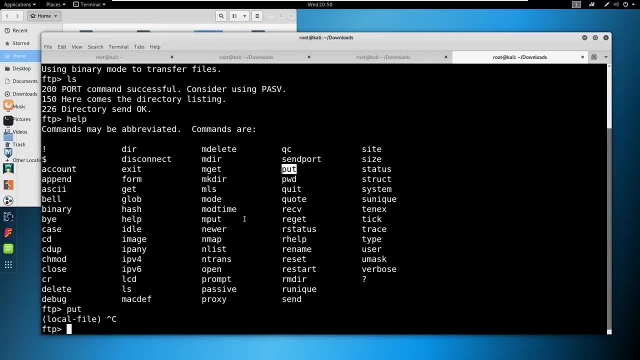 But Sorry, Trying to read the chat and do both, You guys are crazy. How often are versions reported accurate via NMAP? Pretty often accurate, But anyway. so without a way to target this right now, you know, unless I can get a user to open up an FTP, you know it's still bad that I can anonymous log in. 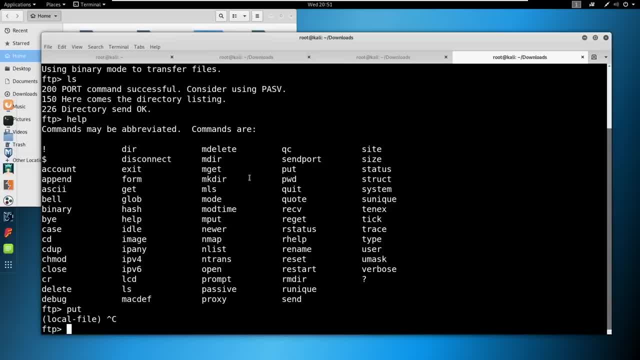 This is definitely a finding on an assessment. But unless I can social engineer a user to open up some mouse, This is definitely a finding on an assessment. But unless I can find a way to execute that malware that I put in, it may not be worth my time at the moment, unless I can find a different way to execute that malware. 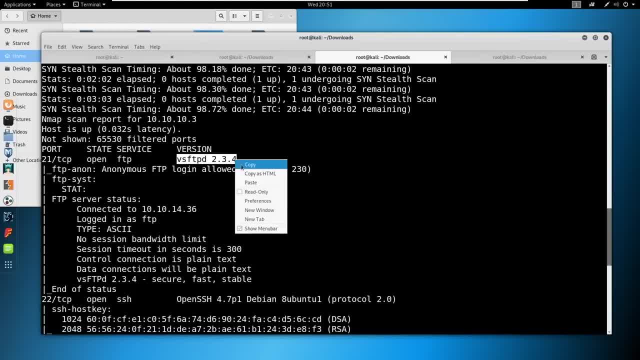 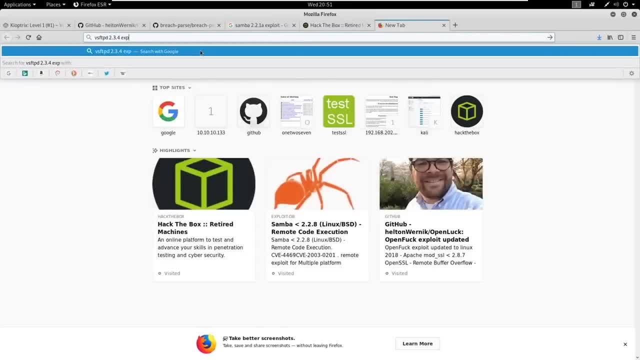 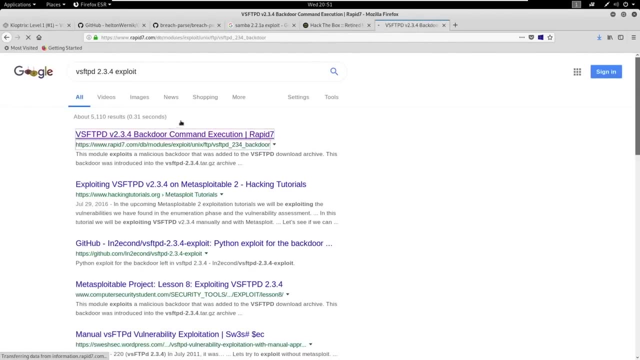 So we can check out this version of 2.3.4 and see if there's an exploit for it. OK, so it's got an exploit for backdoor command execution. We'd go in and we'd read: that Looks like a rapid 7, meaning a meta-disploit module. 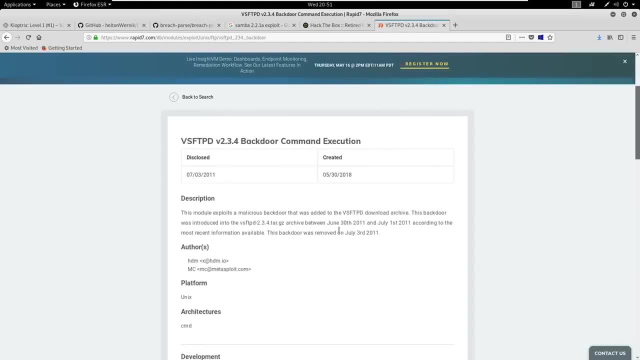 Module exploits malicious backdoor that was added to the download archive. So if this is patched, it's not going to work, And I can tell you right now that it's patched. However, would I be trying this exploit? Yes, I would. 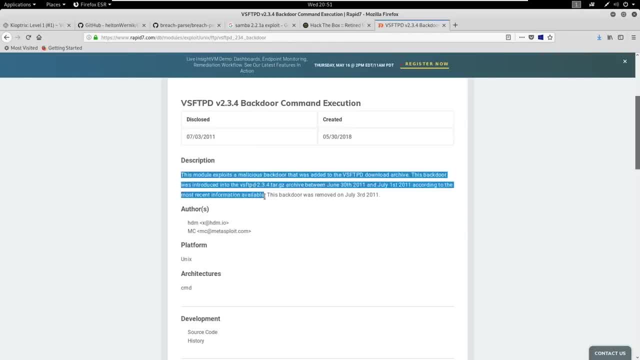 This is probably one of the first things that I would try, But for the sake of saving time here- because we still have another lesson to get into- I'm going to go ahead and just touch on this And I'm going to tell you this one's not it. 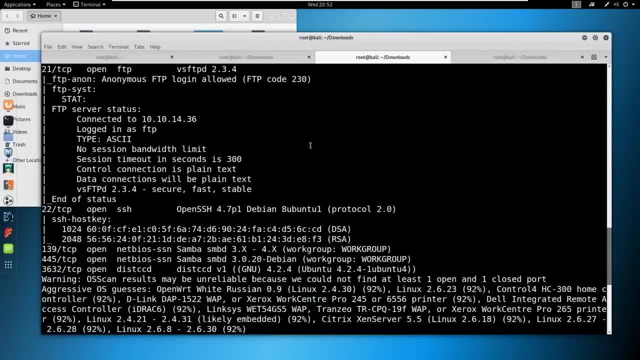 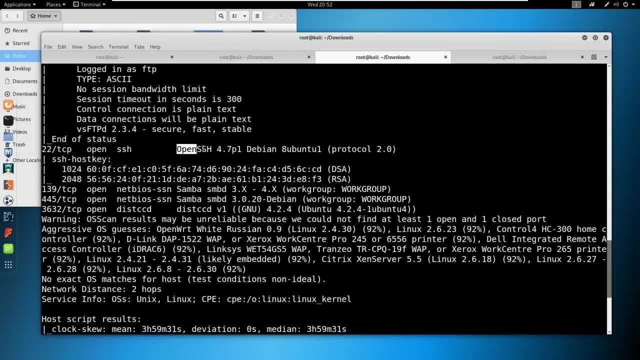 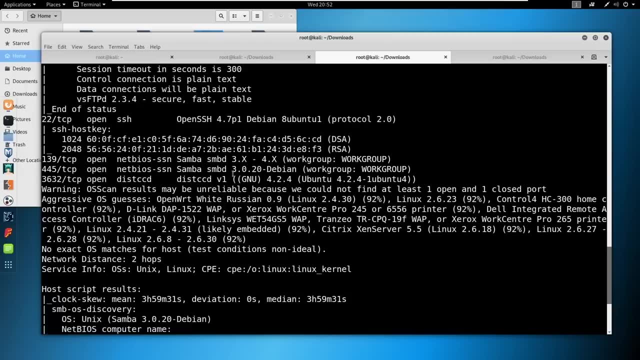 So with that out of the way, SSH I usually don't touch until near the end. I would Google this open SSH and see if I can find anything. But I would also look at this: SMBD 3.0.20.. 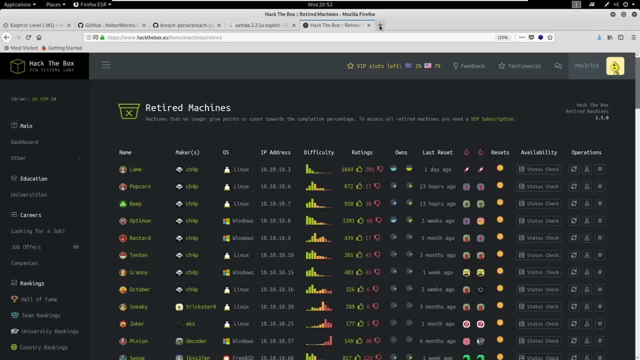 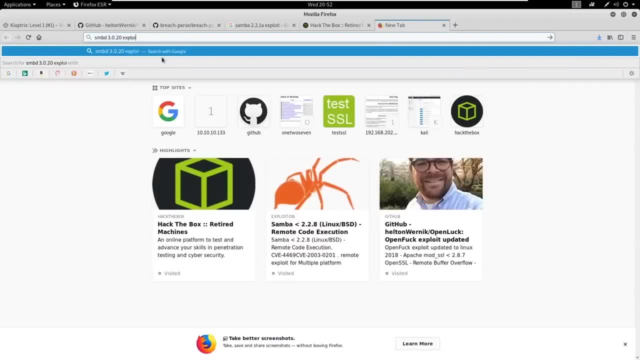 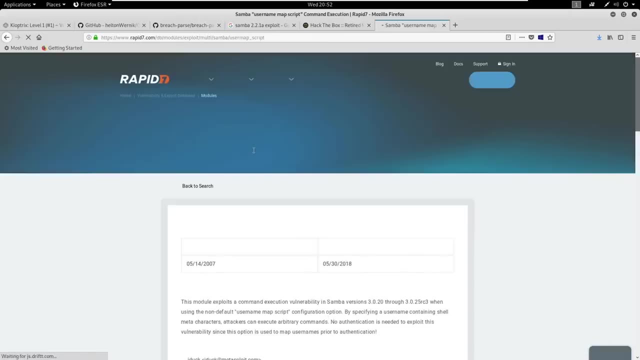 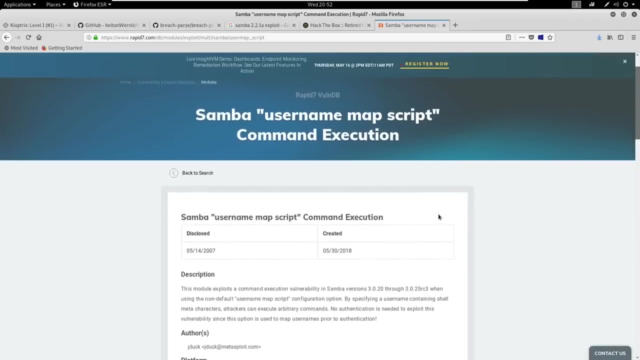 We can copy that, search it And say exploit. I'll just take that off Debian and say exploit. Rapid 7's got another one called the username map script. If you guys spoil any Game of Thrones or Endgame for anybody else, you get the ban hammer. 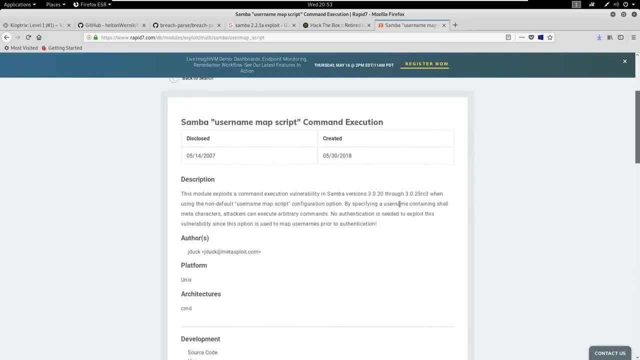 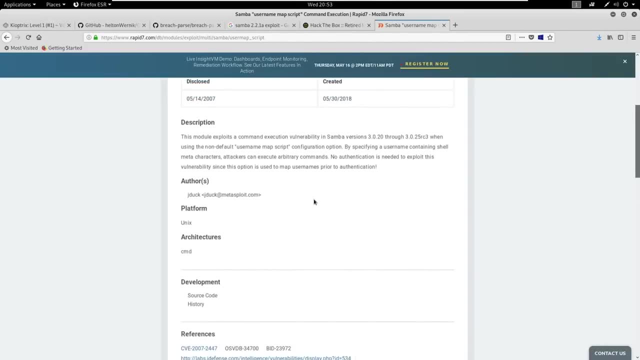 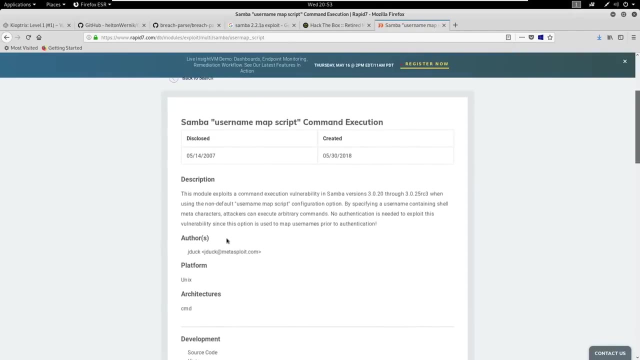 That is just a rule That falls under rule number one of don't be a dick. Also, rule number two might just turn in to stay humble. Just so you guys know. This module exploits a command execution vulnerability in Samba version 3.0.20 through 3.0.25 RC3. 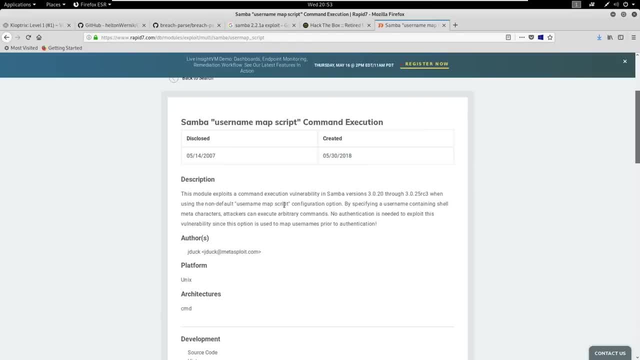 when using the non-default username and map script configuration option. By specifying a username containing shell meta characters, attackers can execute the command. No authentication is needed to exploit this vulnerability, since the option is used to map usernames prior to authentication. This is an unauthenticated RCE remote code execution. 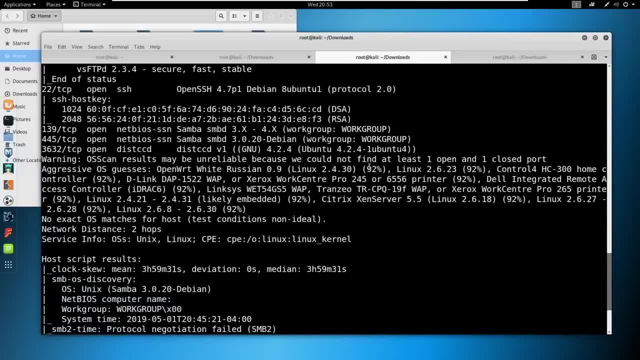 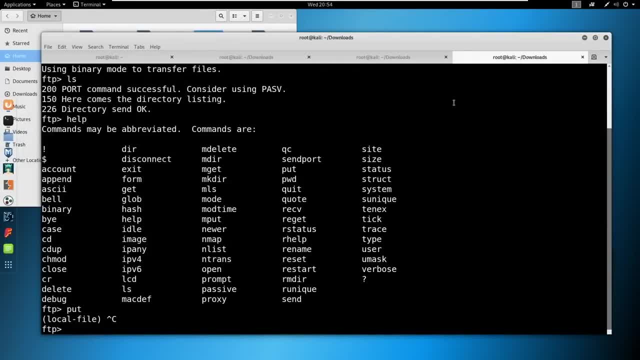 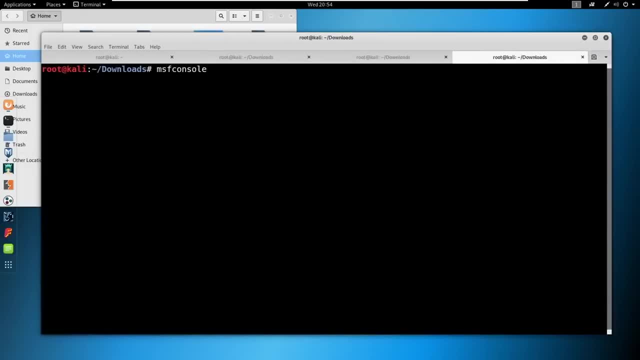 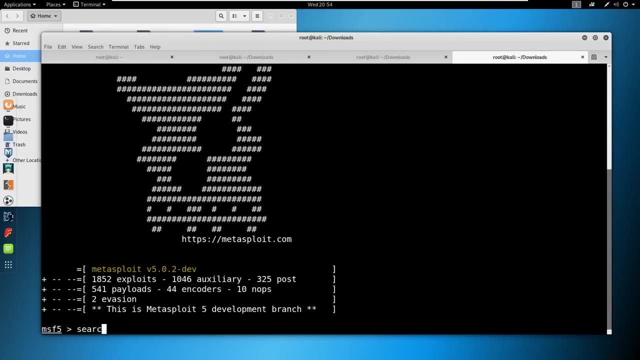 So we're going to try that one Again. this was a username map script, So we're going to come into Metasploit. Well, let's open up a new Metasploit. We're going to search username map. 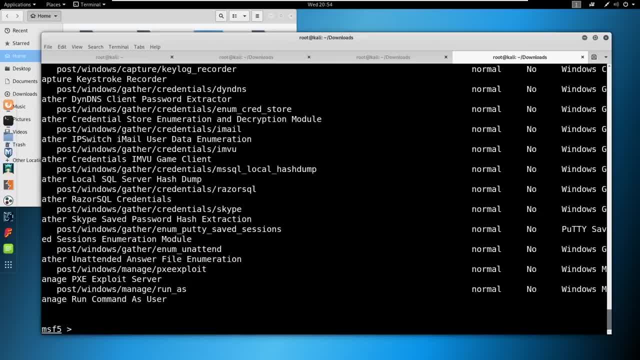 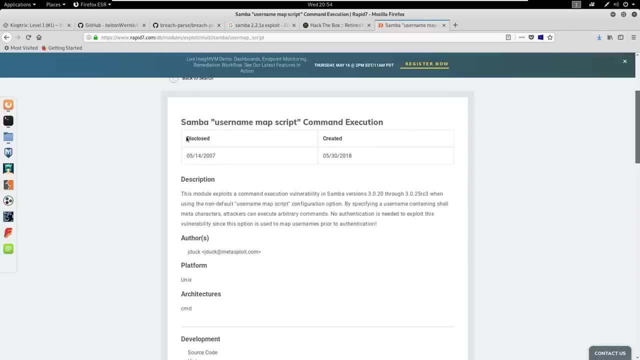 That didn't work. Let's see I'm going to cheat. I don't want to look for it. It's user map. This is why you make notes, And it probably would have told me in here if I would have read a little harder. 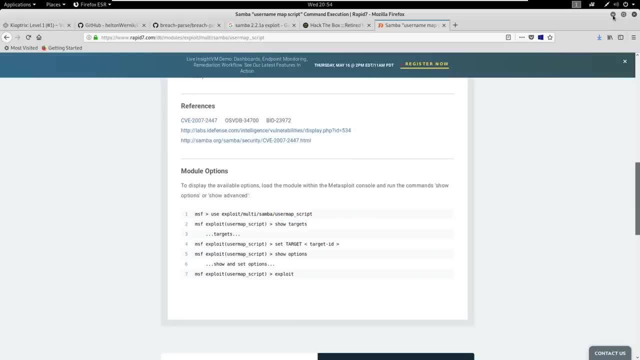 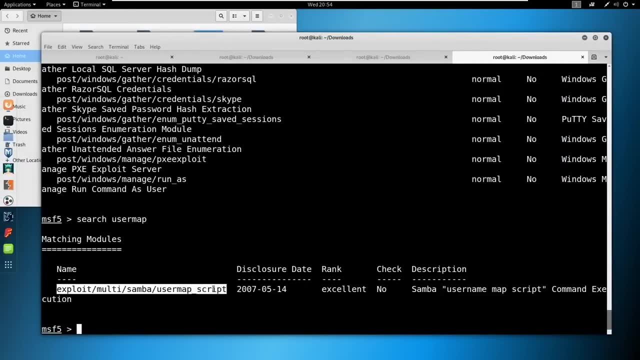 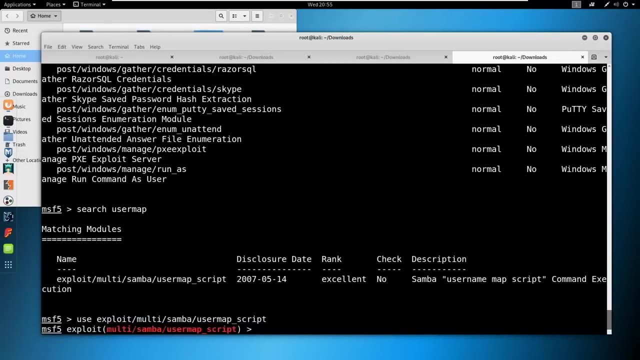 Yes, it does. User map script right down here. Bye JDelta, Bye JDelta, So we'll copy this again. Paste it. We can info, but we already read the info, So we'll just say options. 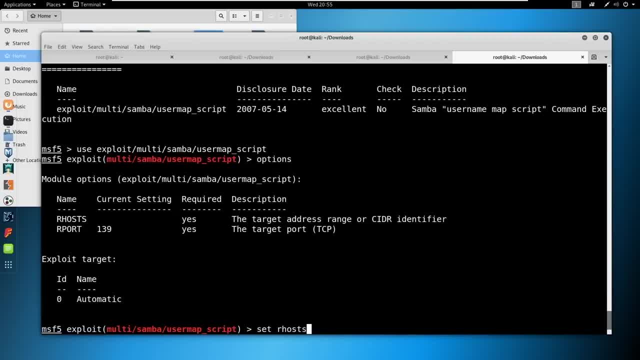 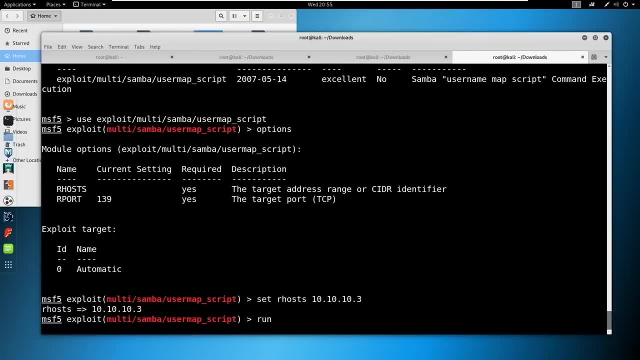 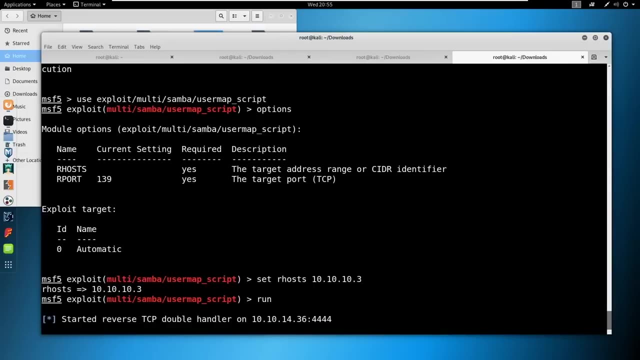 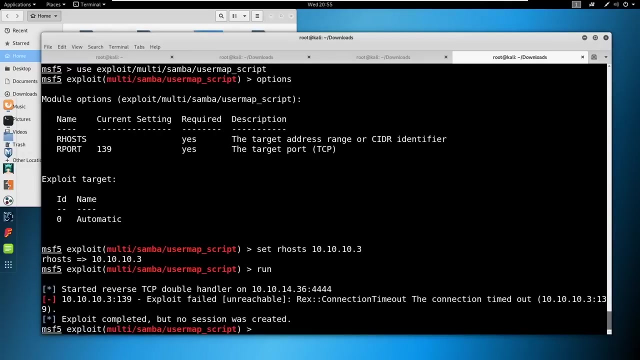 We just got to set an R host, So set the R host to 10.10.10.3.. And the target's automatic, So we'll just go ahead and try running it. Okay, Just going to go to the R host. 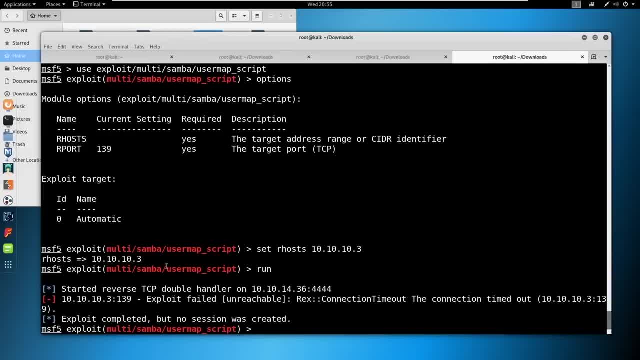 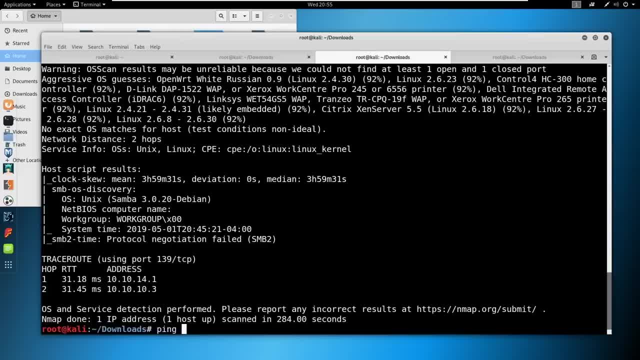 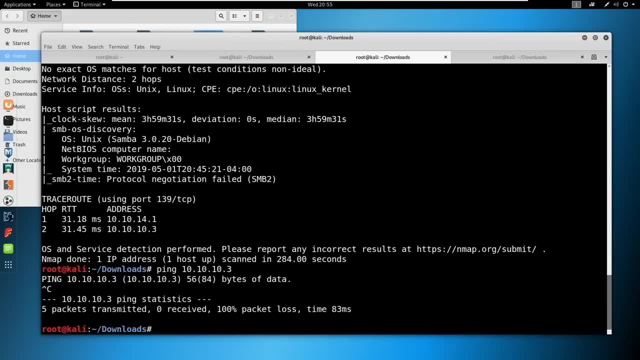 Let's see if it works. Let's see if the host is still up. Let's see if the host is still up, It's not because it hates us. I wonder if our reset just went through or if this box is just incredibly unstable. 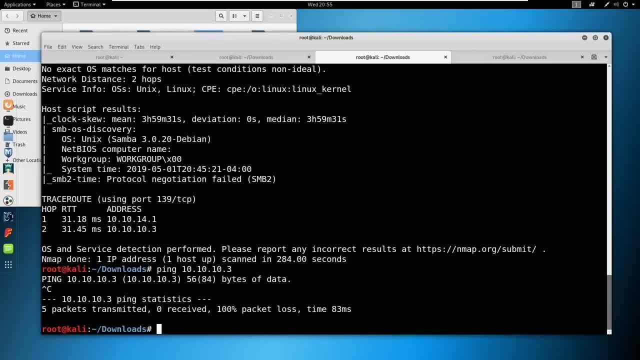 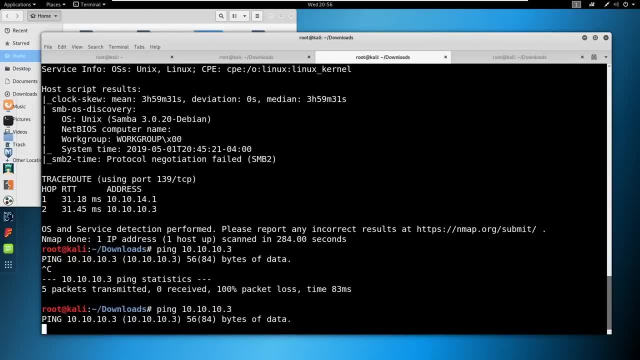 Yeah, this is classic. This is what you pay for. $13 a month. This is what it gets you, So we'll let this run for a second. If this doesn't work, we're stopping at 9 o'clock. I do have VIP. 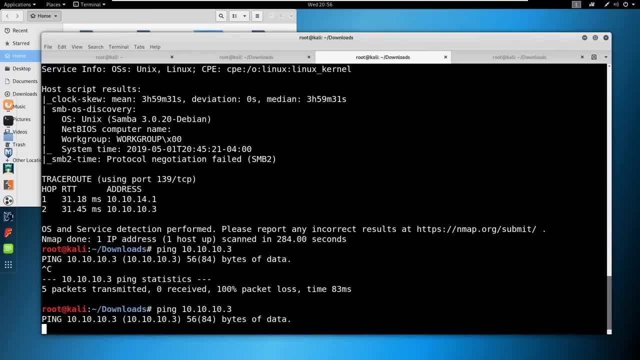 VIP costs like 13 bucks a month. How often do Metasploit modules work for me on tests? Usually often if I'm confident about it. but you know there's some like, like you saw the VS FTPD right, I would have been fairly confident that it was working. and or if that would have been, 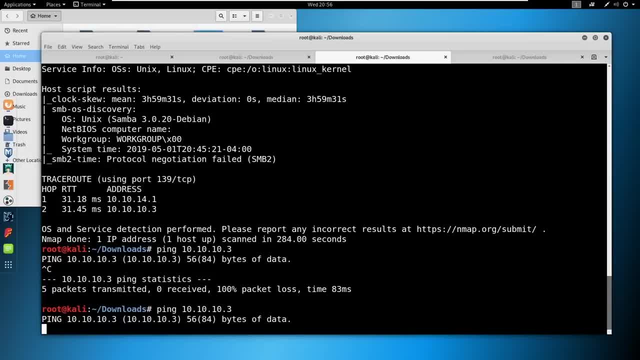 an exploit. I would have fired off and it wouldn't have worked. It didn't have the backdoor version in it. So you run into situations like that. There's some where you're just like: yeah, I know, this is money. 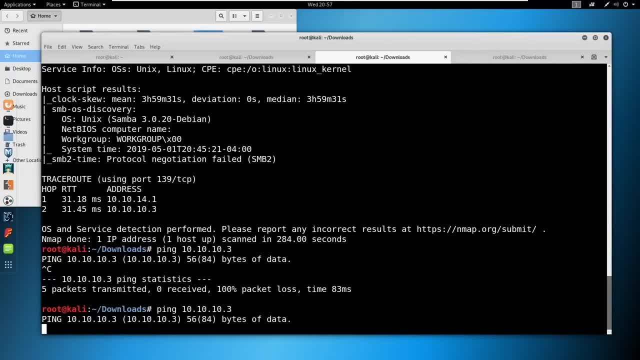 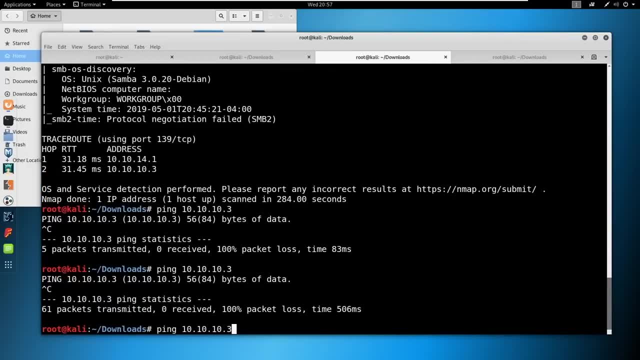 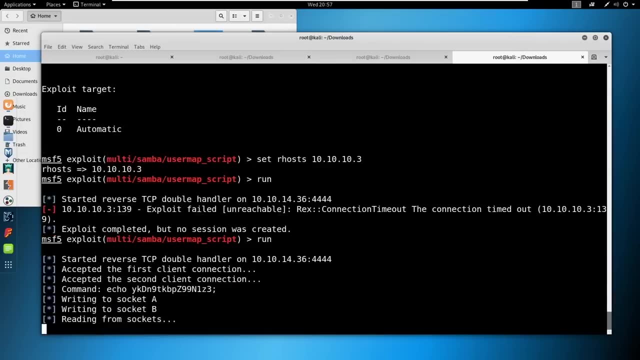 It's going to fire it off, It's going to work. But sometimes you do have to To kind of spray and pray, I guess, to the best of your abilities. There we go, All right, run And we've got a shell. 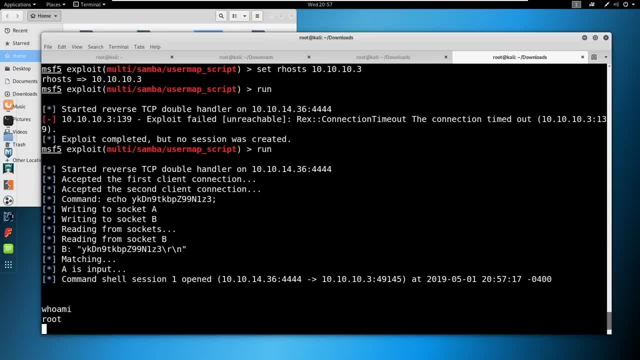 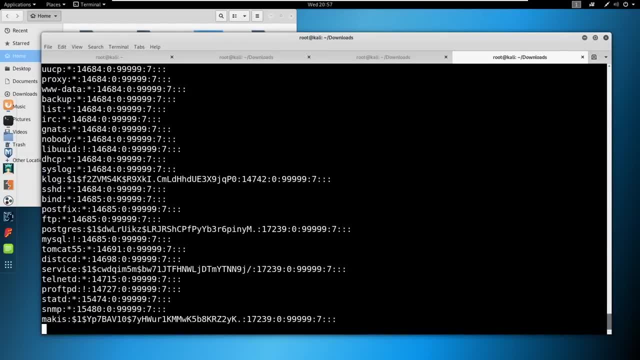 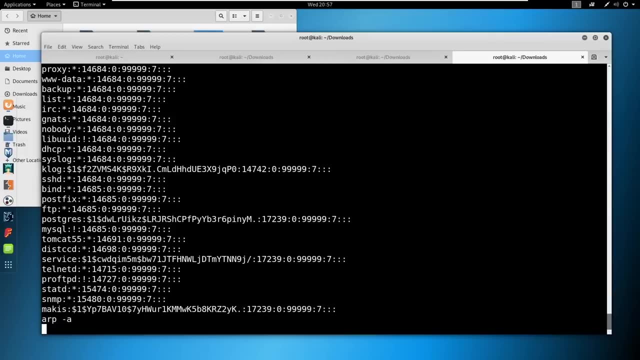 So again, who am I? We are root. Host name Lame. I would cap the Etsy shadow. again, We are root. We can steal all those hashes in there. We can ARP dash a if it responds back in an orderly fashion. apparently they don't. 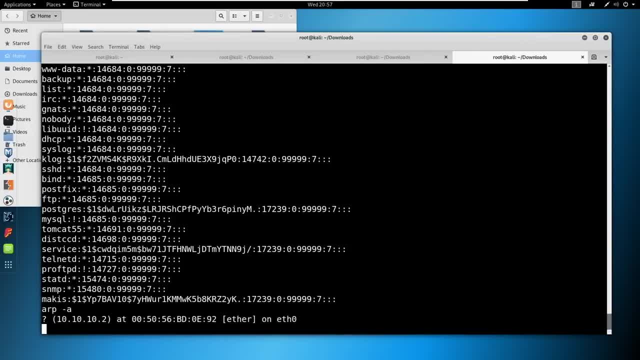 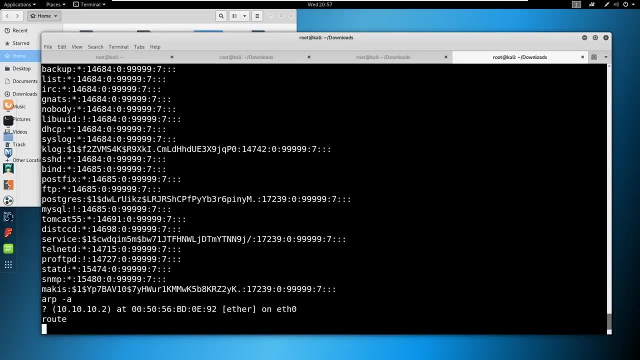 like networking commands today. There it is, We can print the route. If I was a low level user, pseudo dash L: Yeah, Yeah, On a scale this fast, do we go that high? Yeah, I think so. Let's put it at the top. 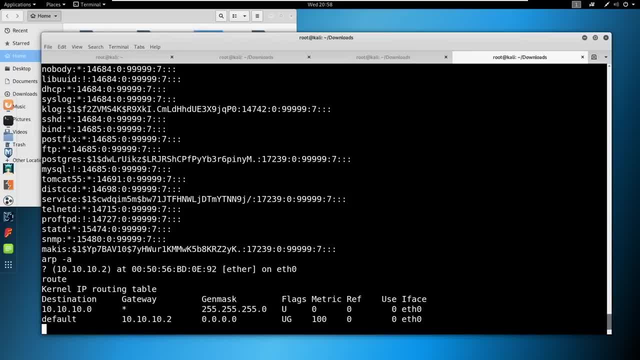 Yeah, Yeah, Yeah, Yeah, Yeah. Actually, that's a great idea. Let's take a look around and see what actually happens after that. If we need to do that, let's take a look at the security code. So we don't even go to the security code. 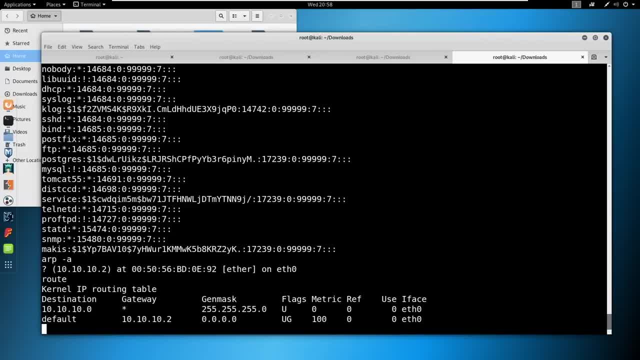 Now, if we want to do that, we go into the security feature. Then we can tell this is the password and then we can just type in the password. Oh okay, We have the password. And then we can say: check. 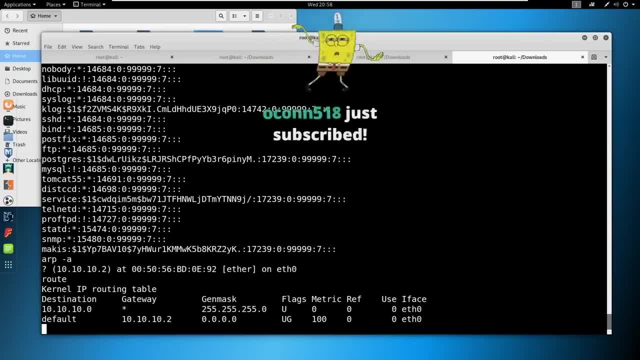 All right. So in this case we want to have the password to the passcode, So we're going to use the passcode slash L. Again, I would look around for important, definitely look around all the the files that i could find and see what's interesting in there. 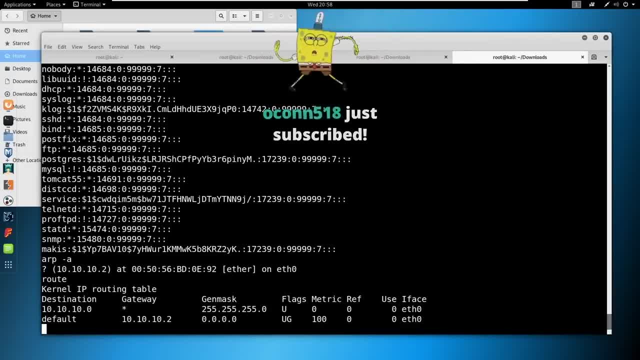 um, that's really what enumeration is right. if you're meticulous and outside, you got to be just as meticulous on the inside, especially if you're doing capture the flag stuff. uh, thanks, okan for the the sub. i appreciate that. oh, thanks all you guys. thanks immunet, thanks. low kids appreciate it. you guys are awesome. 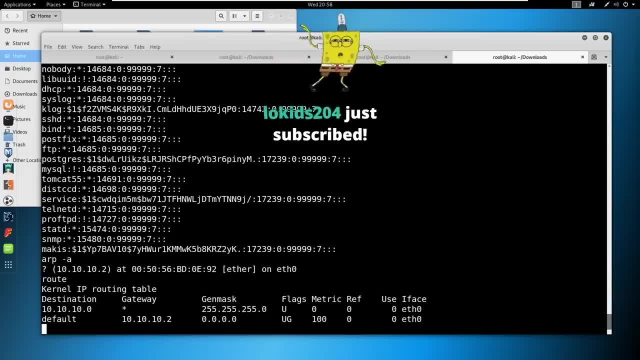 okay, so that is it for exploitation. we are running right on time now. if you are on the mailing list, uh, you notice that i sent out. but we're gonna be talking about what do we do in a situation where there is nobody that or nothing right that we can exploit? uh, let's, let's, even. 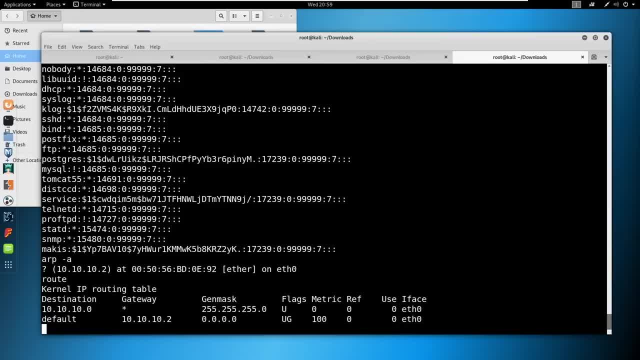 narrow this down a little bit more, because some of you are going to jump right to social engineering. well, i'll just call the help desk and tell them i'm so-and-so and get the password set. yeah, that's possible, right? uh, you can definitely social engineer, but with a lot of these engagements, a lot of pen. 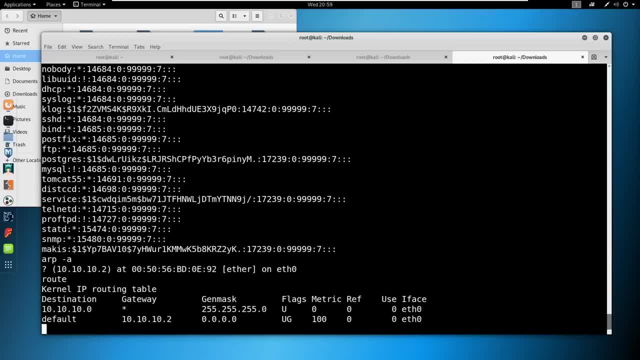 testing. external network engagements have no social engineering allowed. there are different types of assessments for that, sorts of assessments for that. where there are full-on engagements that allow social engineering, they're strictly social engineering engagements. so companies like to limit you in scope as much as possible. humans are the only ones that can do that. so you can definitely social engineer, but with a lot of. 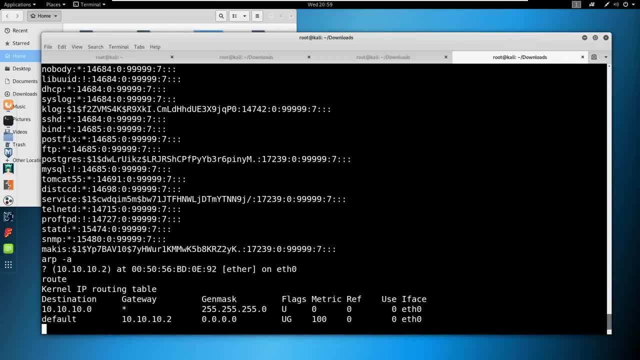 the weakest link and we can still exploit humans being the weakest link, even if everything else holding true, uh is pretty much unexploitable. right, say, this company's up to date on their patching uh, they you know. maybe you find some small vulnerabilities, but there's nothing that. 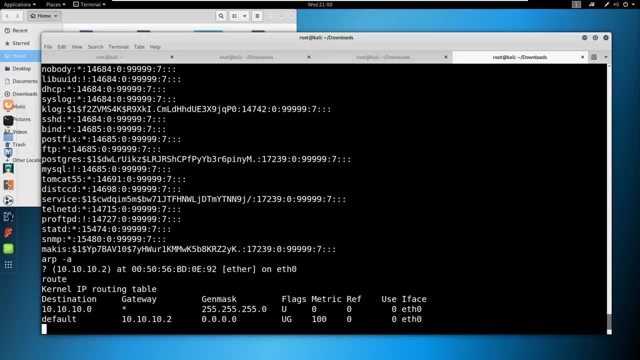 you can get remote code execution on. that's what we're going to talk about tonight. now, if you sat through my carolina con talk already, this is going to be semi-repetitive. um, but only a tiny piece of it is from that carolina con talk. so, uh, somebody asked about the website. i'll pull up the. 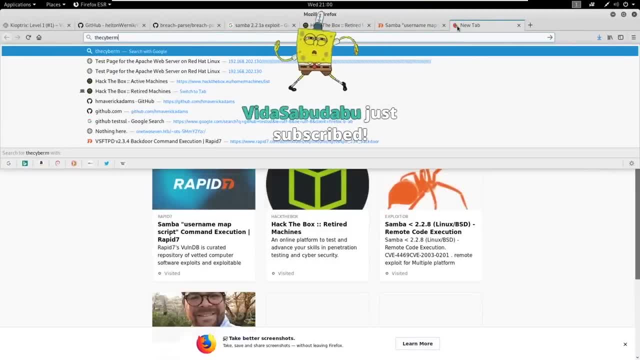 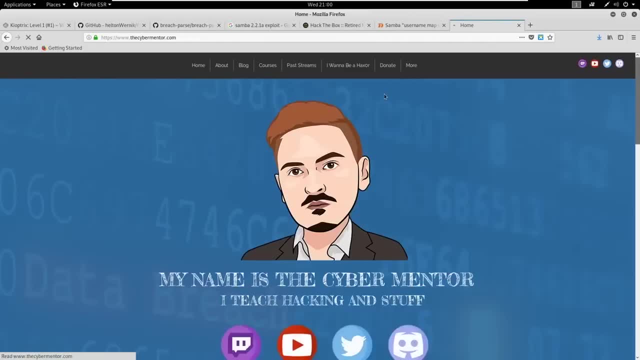 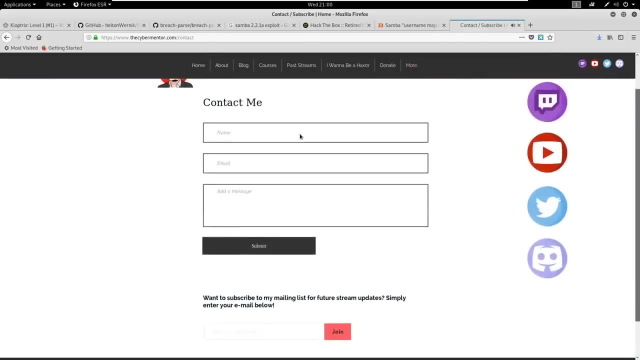 website really quick if you want on the mailing list. thank you, vita, i appreciate this up if you come into- oh, there's a more up here. okay, you come into more the contact subscribe and you come down to here. this isn't the best website. i'm not a good web dev. 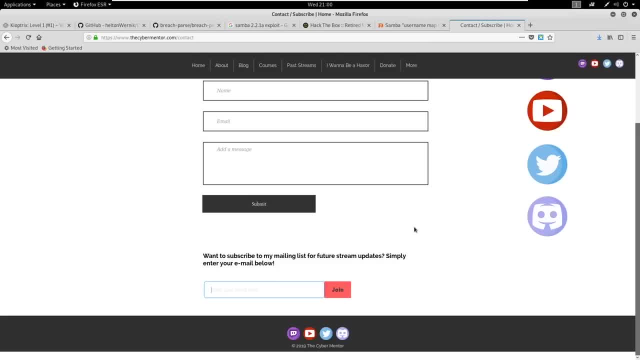 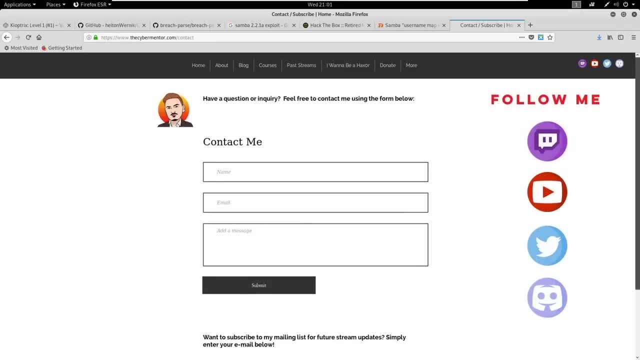 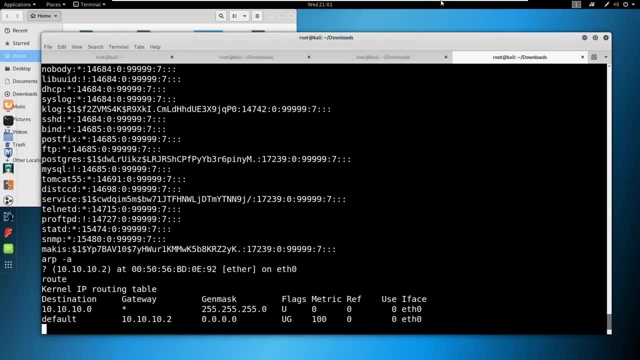 but if you come down here and just join the mailing list, you'll get the weekly email. all right, so let's go ahead and talk. did i draw my logo? no, i didn't. i bought it on fiverr because i'm cool. if you're not getting the emails, i would try resubscribing. 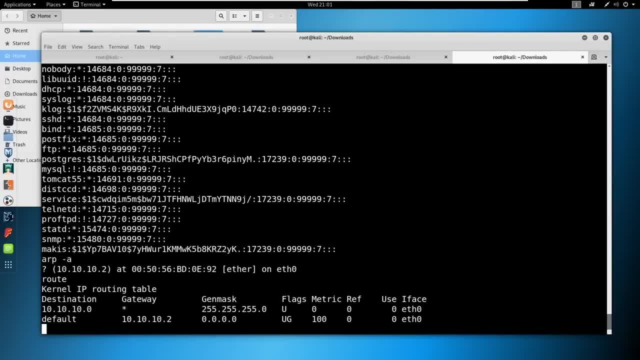 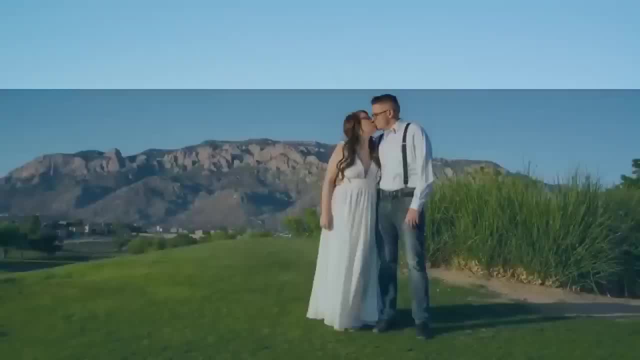 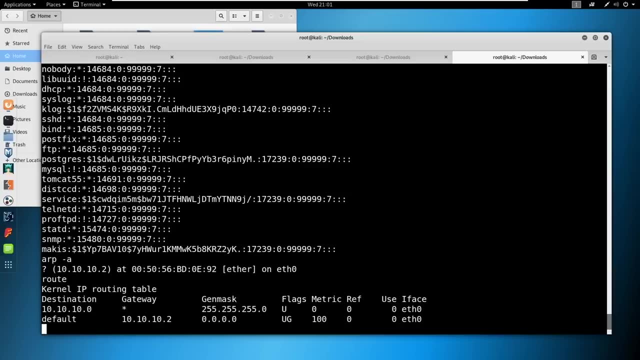 you might have typed in the wrong email. fiverr is dope. all right, let me get up this powerpoint presentation, since it killed my original one. so we're going to talk about a couple different concepts tonight, and we're going to talk about- uh, we're going to be talking about- credential stuffing and password spraying. are 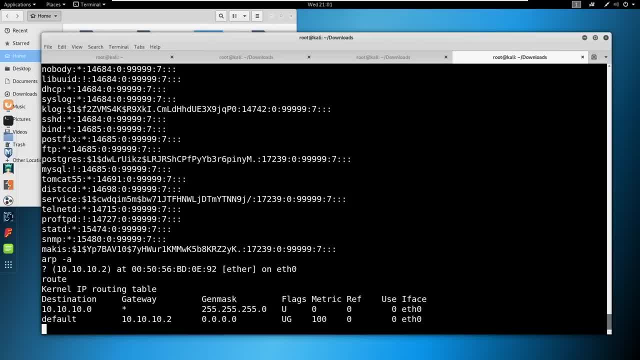 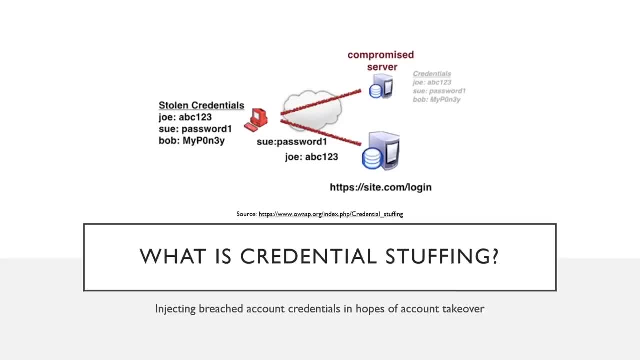 some of the biggest items that we can do when social engineering is not allowed. so let's go ahead and present this from the current slides. you don't have to go through my whole spiel again. all right, so we're going to start off with credential stuffing and then we'll talk about password. 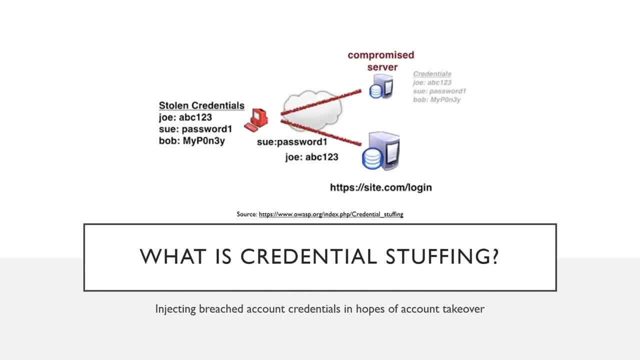 spray. so what is credential stuffing? well, it's injecting breached account credentials in hopes of a takeover. so we've got a compromise server here, right, you see the compromise server. we've got credentials for joe, sue and bob. these are part of some breach. you can think equifax, you can think linkedin. 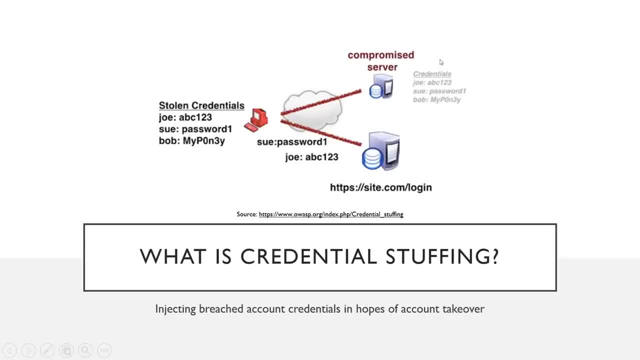 you can think, whatever breach you want, these hashes get taken. people take the hashes and they take them offline and crack them for you. sometimes they're nice and they put them on the clear web. sometimes they put them on the dark web and try to sell them. uh, so, however you obtain this, you can get these clear text passwords. ah, joe's up here, we got joe. 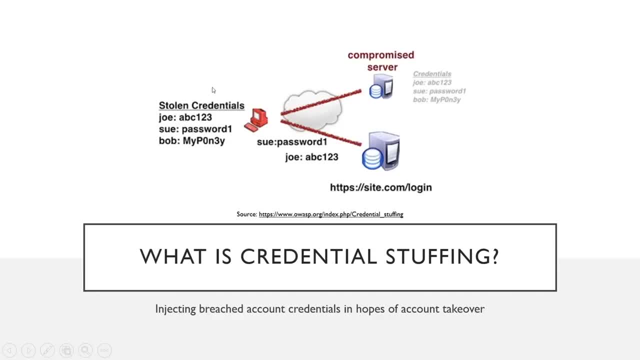 god damn it, joe. we take these, these clear text passwords, right and we try to put them against website logins. if you're a bad guy, you're putting these credentials uh, firing them off at random email servers. you're firing them off at banks. you're firing them off wherever you can log in. 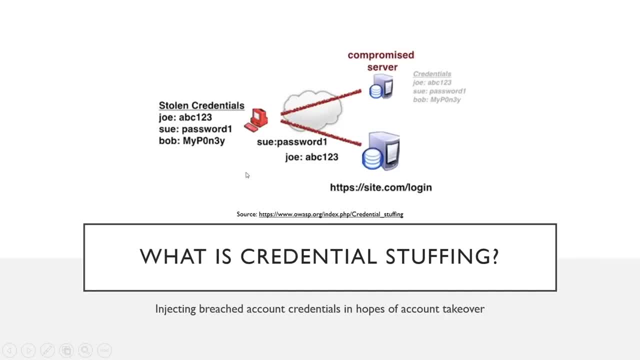 with them, right? if you're a good guy, well, what you're going to be doing is you're going to be staying in scope like the good hacker that you are, and you're going to try to log into a website that is owned by the client. so, and if you're lucky, these credentials will work right. 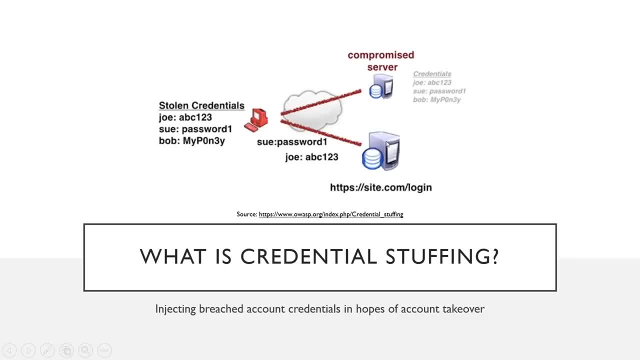 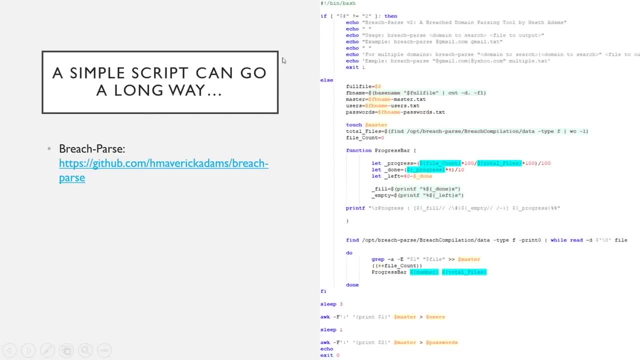 away, and that is the benefit of credential stuffing, so a simple script can go a long way. this is actually version two. we are now in version three, so people have been asking about breach parse. here's the github for breach parse right here. so basically, this tool, what it does is it searches. 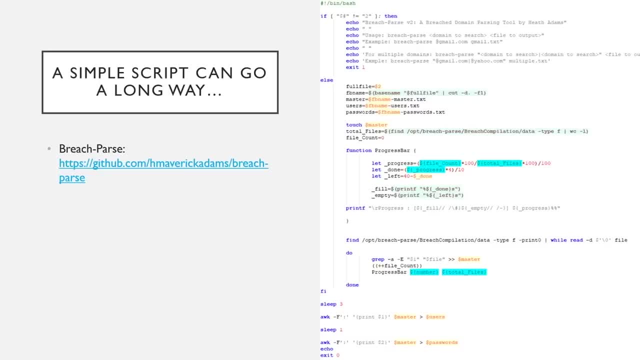 through a 1.4 billion clear text password list and it spits out what you, uh, what you specify to spit out. so if we go through the script really quick and it may be hard to read, basically this is the usage up here. if you see it says breach parse domain to search. file to output: uh, so if you wanted to, 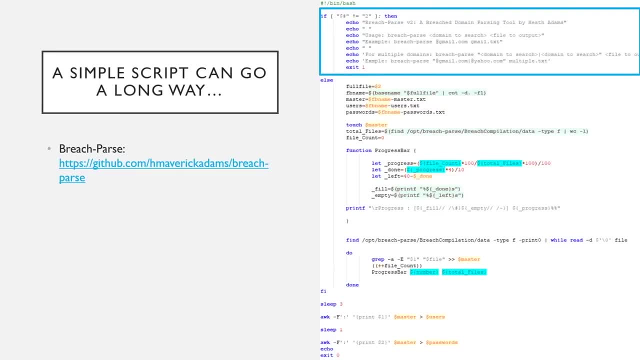 search and we did tesla last week. we're actually gonna do tesla this week again. we're just gonna keep with tesla. if you say breach, parse at teslacom and then just say teslacom dot text, it'll go ahead and output that for you. uh, so what it's going to do is it's going to roll. 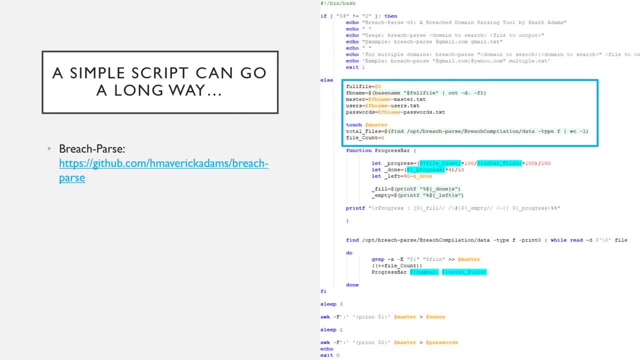 through and it's going to create a bunch of files. it's going to create a mastertxt. it's going to create a userstxt and a passwordstxt. now the mastertxt has a username colon, password- users is just all the users, passwords is just all the passwords. that way you don't have to do an awk and 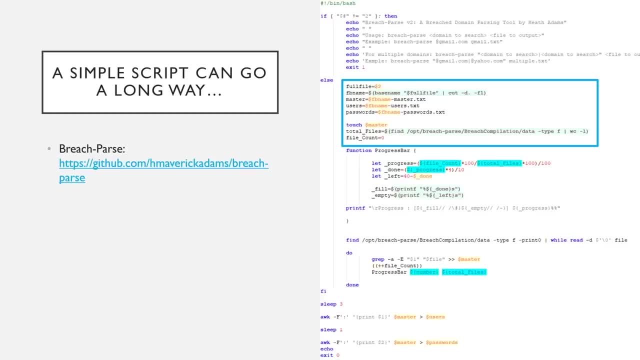 sort it out. i'm already doing that for you. uh, so we do it for you. and then we're going to go ahead and touch of a master file, we total all the files and we do a file count because we build a progress bar out here with a function. uh, basically it's just so we know how far along we are, because i 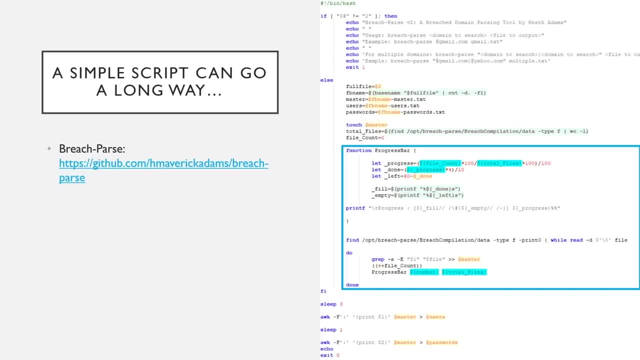 got tired of watching this roll through and not knowing where it was at. uh, so has the function of the progress bar. more importantly, all it's doing is doing a find command. uh, it's finding what you put in there as that at teslacom. it's looking for at teslacom through every single. 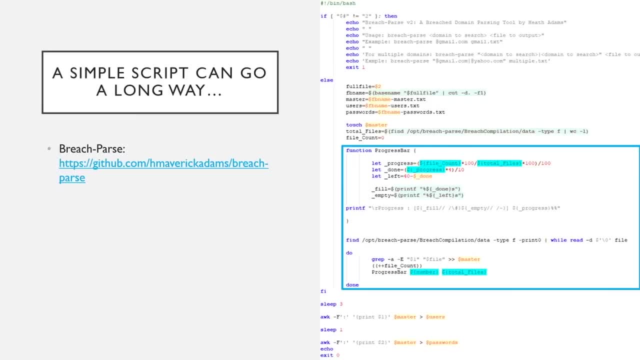 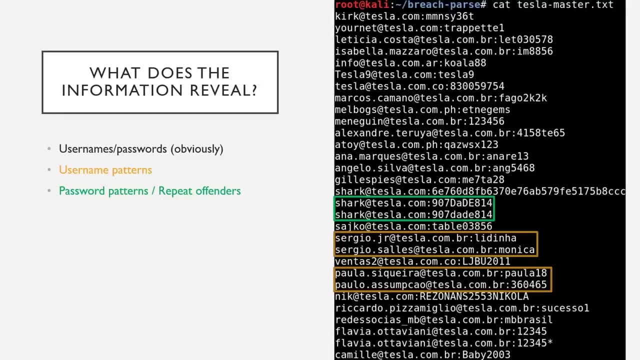 file that we have and when it finds that it greps or it looks at the files, then it greps for that and then it outputs it to the master. from there, the master. we output that to users and to passwords via an awk and that's it. it spits out something kind of like this: so you're looking at the tesla. 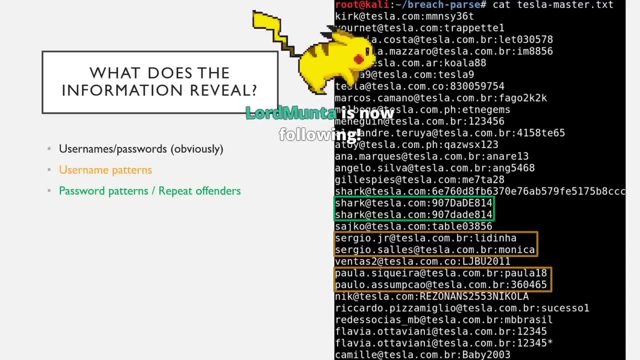 dash mastertxt. uh, you can see a few different things here. so what does the information reveal? reveals, obviously, the usernames and passwords, right um. but also it reveals, if you look at the orange, it reveals the username patterns. so you could see that sergiosalez or paulai can not. 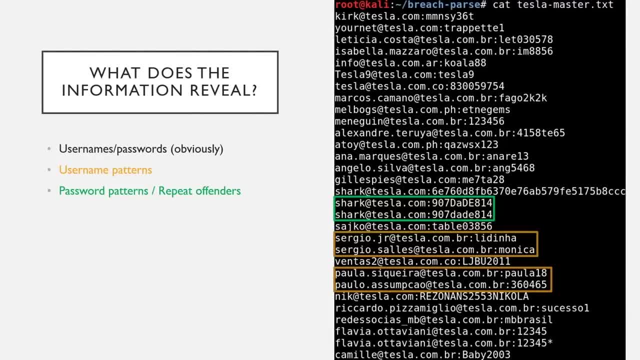 even pronounce that. uh, you could see that there's a first name dot. last name now for tesla. this does not hold completely true, because you see some first names in there as well. uh, you see kirk, you see camille, and it's probably under assumption that what happened was. 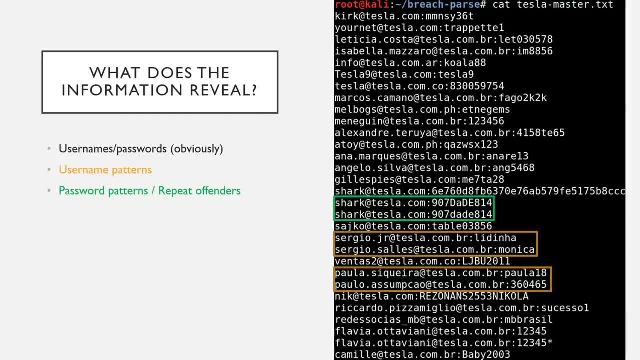 maybe when they were smaller they had a kirk, but as they grew bigger into the large company they are, they had to start moving towards a first name, dot, last name, and i've even seen first initial last name now, so they may have changed their email a few times over. on top of this, there's 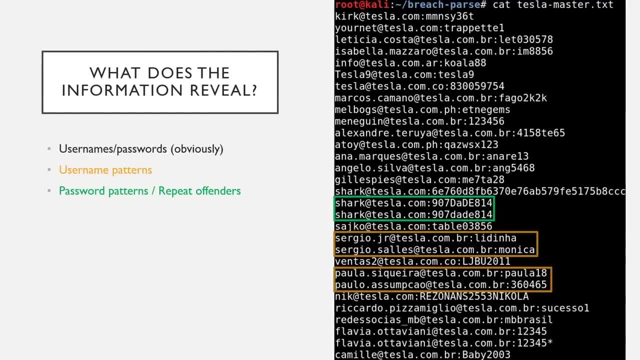 some other information that we can gather here. we can see password patterns and repeat offenders. so with password patterns and repeat offenders, we're seeing the shark at teslacom. this person's shown up three times. one thing that's really really interesting is this password right here. 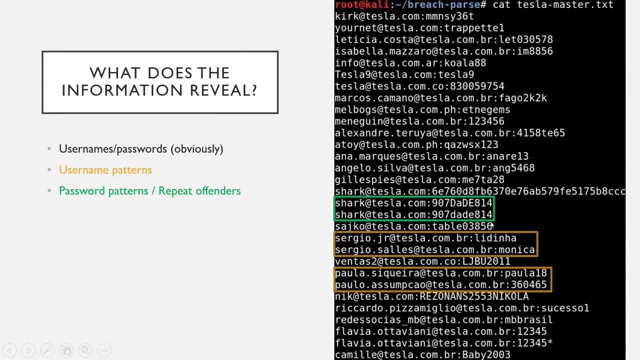 where you see the 907 d-a-d-e 814. so you see that they just changed the rotation of capitalized letters and non-capitalized letters here, so it doesn't really. i mean, it gives us, you know, x amount of possibilities, right, but it doesn't really give us a lot of possibilities, right. 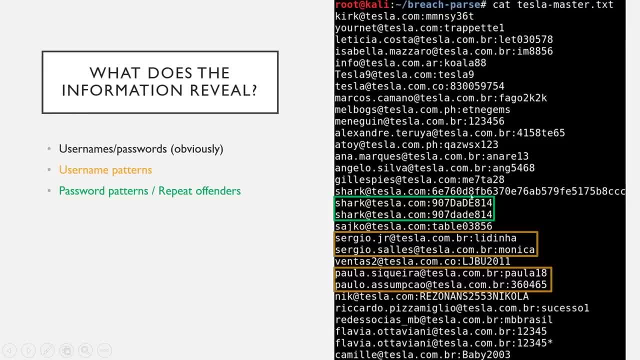 but in a four character space with capitalized letters and we're holding the rest constant. i can run through something to to make all of these out and figure it out pretty quick. so when we look for patterns like this, we may be able to easily hack into a company that has poor. 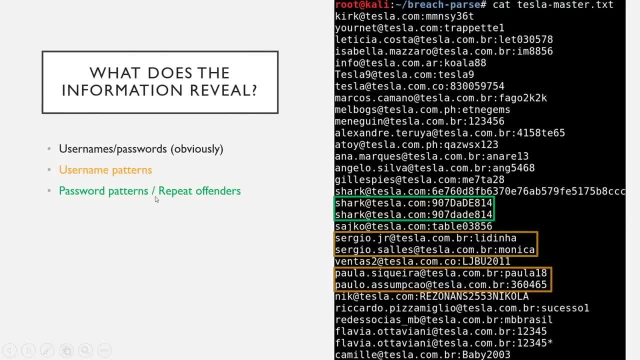 password rotation, and there's some more advanced thoughts here too that i don't actually have on this slide. if i'm a bad guy or i'm doing a social engineering engagement, a full-on red team engagement, what i might do is i might take this password, this 907 d-a-d-e, or let's we 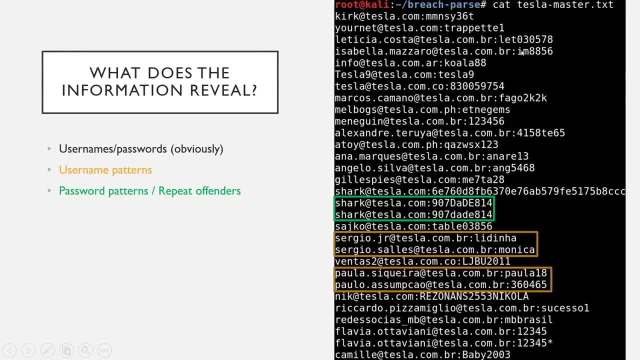 can find one that's even more more complicated. i think this one's probably one of the better ones on here. uh, maybe trap that one as well. uh. so what you do is you say, okay, i want to take this 907 d-a-d-e and i'm going to take it and i'm going to put it back into its original hash format. 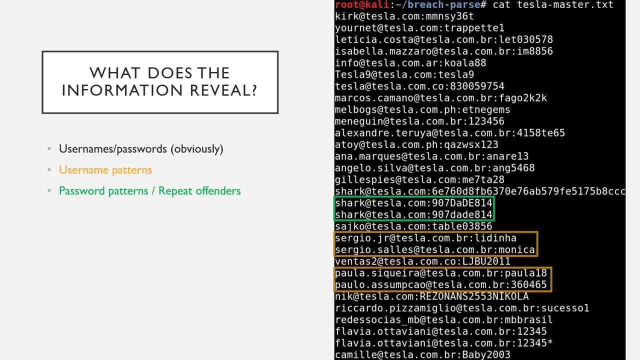 we don't know what original hash format it was, so we'll probably put it into like four or five different hash types. we'll take those hashes and then there's sites like unhashed that you pay a small fee and you can run it against a hash table. 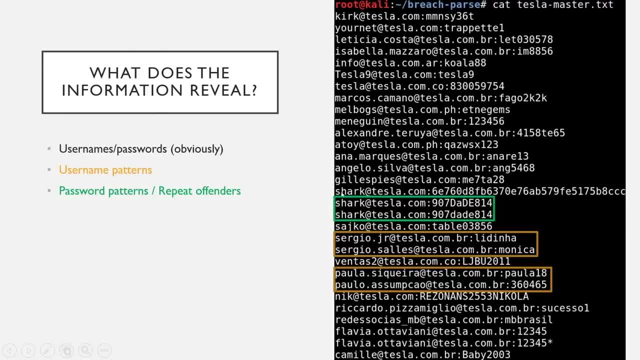 and get the email address tied to that. so what does that do? well, one, it finds the hash for a password that hasn't been cracked yet or isn't a part of these lists. just because it's crackable doesn't mean it's been cracked, uh. what it also does is it ties some of 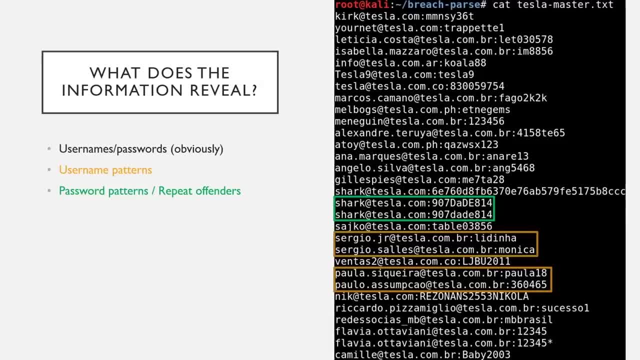 these hash types together. and then it finds the hash that hasn't been cracked. yet more unique passwords to almost a more definite user right. if it was password one, okay, we're not as sure that's gonna. you know there's gonna be so many of those, but something unique like this. 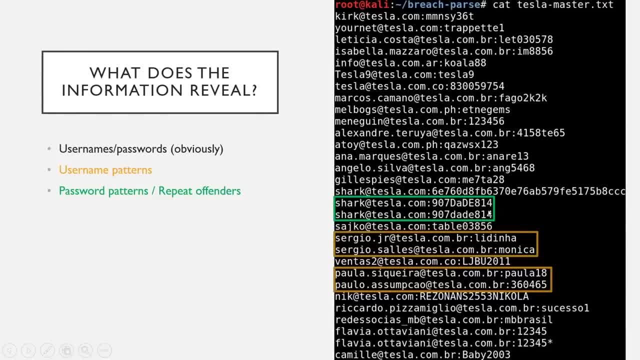 907 d-a-d-e. 814 um. i'm gonna be a stronger confidence level that if i see it pop up and it ties to a hash, or even if i put this string in and i put it in through my clear text list again, right, instead of at teslacom, i'll put it through the clear text list and i'll. 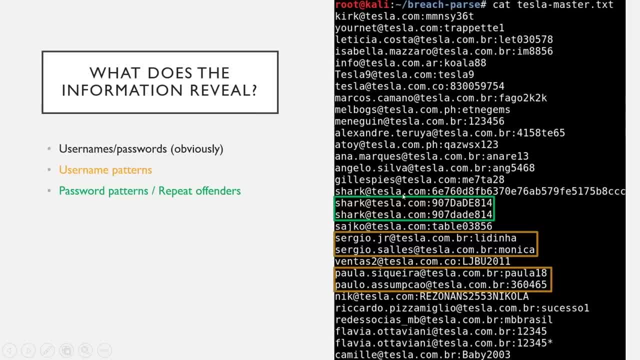 try to see if this comes up for a different email address, so we can really start finding out what websites this user uses and how we can exploit them further, especially if we're a bad guy right, or doing a red team assessment and there's nothing off limits. so you know these, these. 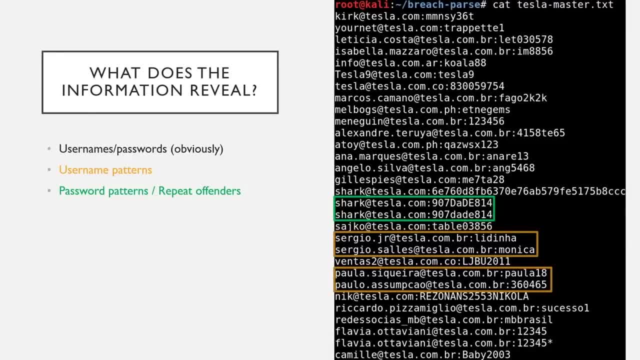 passwords really come into play, and and when people are using their work emails like this, it makes it easy for us to just exploit the hell out of them. so we're gonna do this tonight. this is what we're gonna do tonight. we're gonna do this tonight. we're gonna do this tonight. we're gonna do. 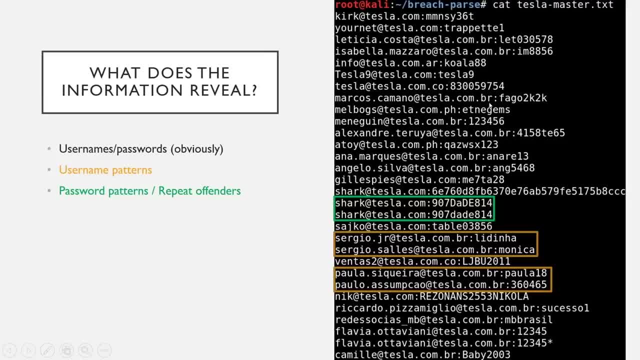 in the last 20 minutes we're gonna do a little bit of credential stuffing. i actually don't even know if there's a login, so we may just pretend, and if there is, uh, if there is no credential stuffing found, we're going to talk about password spraying, and they're pretty close to each other. 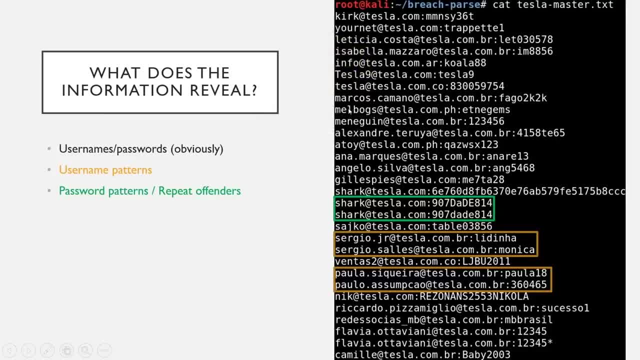 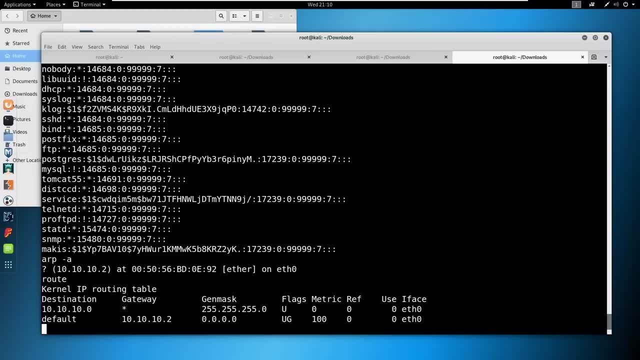 somebody asked: this is when you have nothing else to exploit. yes, that is correct. all right, so let's get out of that presentation. if you are interested in that presentation, you can check out the link in the description below and i'll see you in the next video. 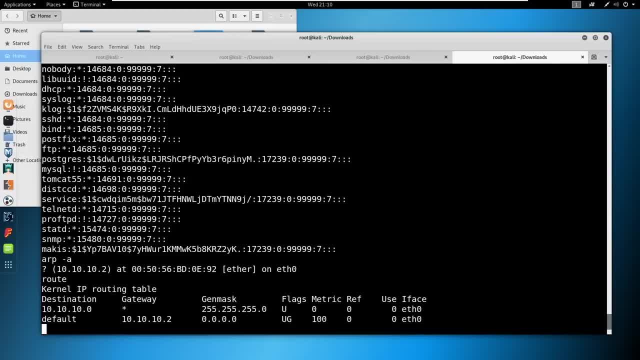 all right, so let's get out of that presentation. if you are interested in that presentation, you can check out the youtube channel. basically, i have the whole thing up there from carolina con, which gives a story of going from, uh, from an external assessment like this and weaving my way in and getting domain. 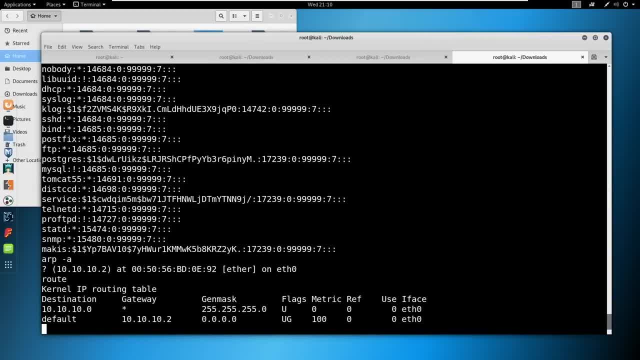 admin. it's a pretty decent story, also covers the blue team side of things. so if you're, if you're more interested, you're welcome to check that out. so if you have already downloaded breach parse, let's go into here and let's just close out everything we're, we're done. 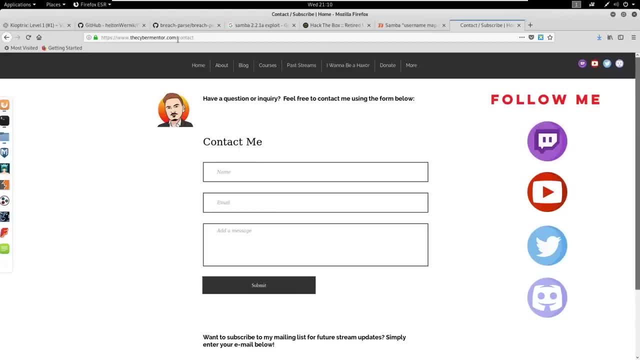 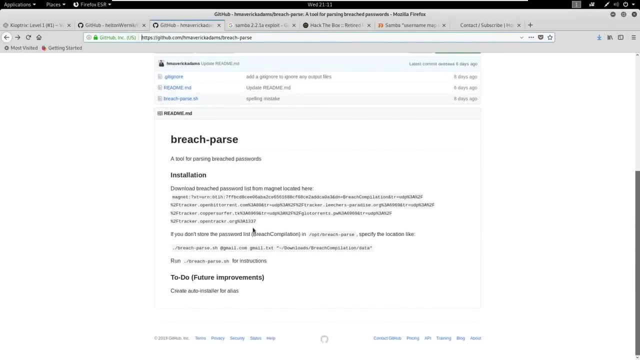 so we come into breach. parse, go back again. we're on version three now, so you have to download the magnet of the clear text passwords. we've gone over this a few weeks ago, so many of you already have this downloaded. if you don't, you're not gonna be able to follow. 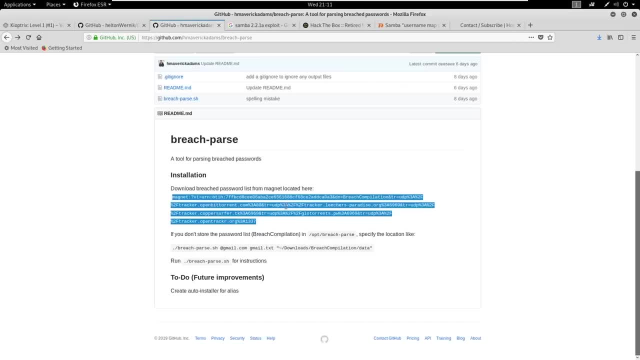 along because this is 44 gigabyte file here. but you will need to download the 44 gigabyte file from this magnet and put it on your machine and you're going to be able to download the 44 gigabyte file from your machine. from there you can install breach parse- the only updates that have been done. 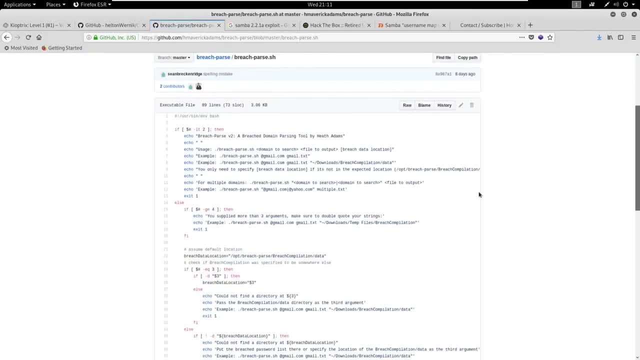 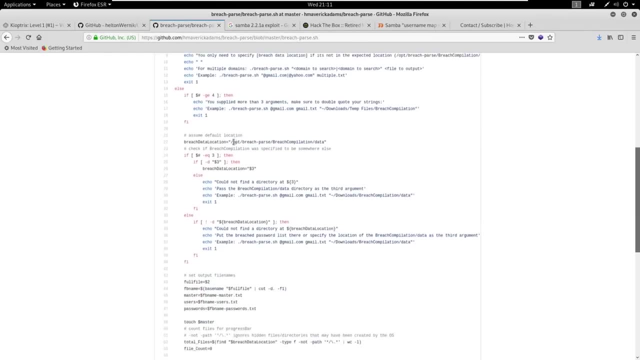 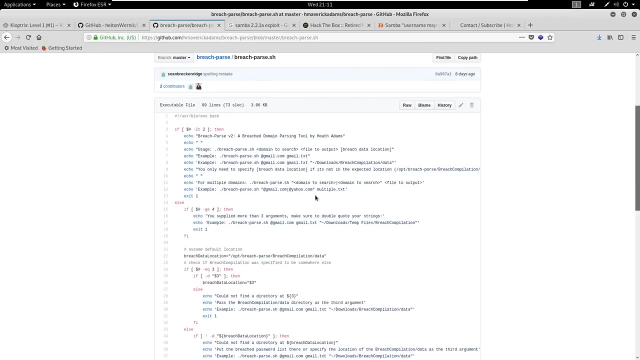 is. we have now the ability to uh to add a breach data location. originally it was hard coded. it still is hard coded here. but if you supply the location as in it's somewhere else other than the opt folder, the breach parse folder, then you can just supply the location of the breach. 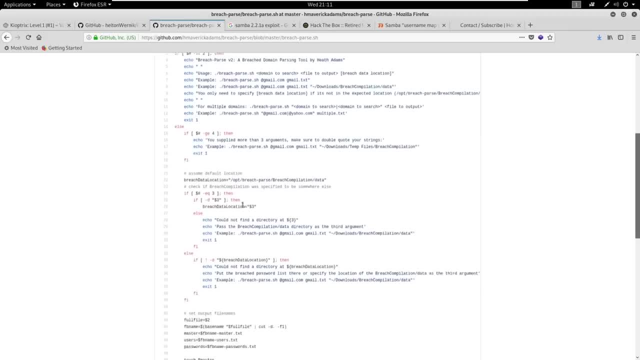 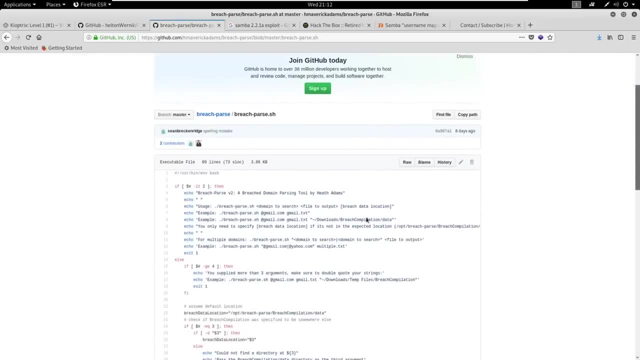 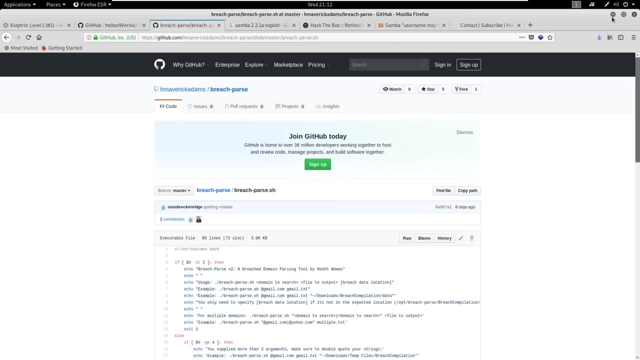 compilation data and search through that area instead. uh, so somebody forked this and did a good job. sean breckenridge, thank you. so it is a lot of gigabytes, but it's a lot of information and it will get you easy win on an assessment. i've gotten so much win on assessments from this. 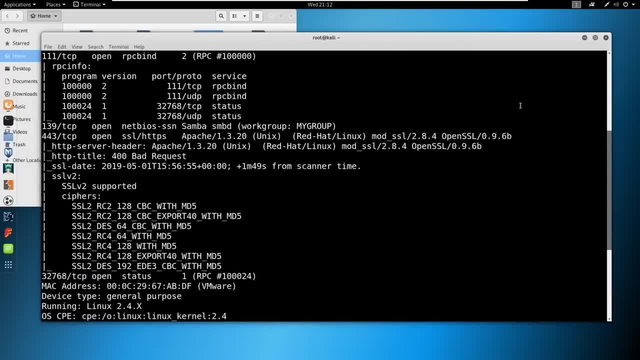 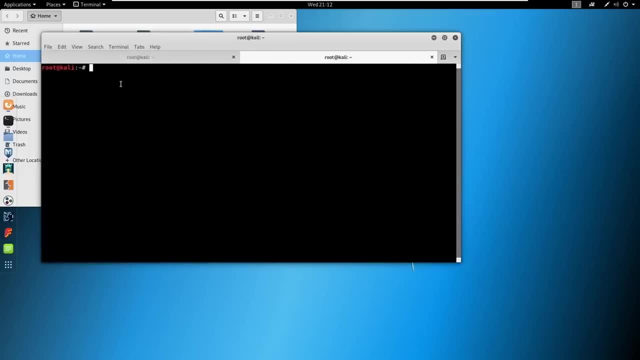 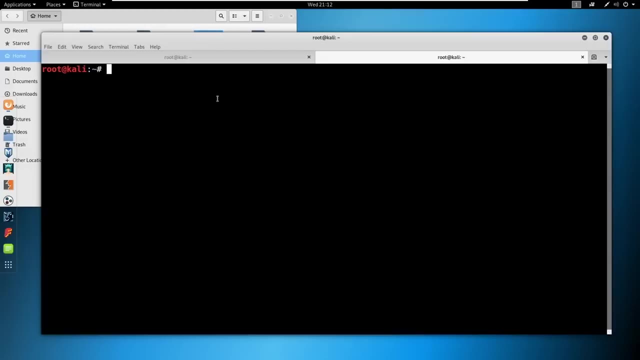 this script came from being flustered and not having literally anything on an assessment that i could have that i could find ended up breaking in with it. so let's go a new tab again and i've got this alias. if you're following along, you can, uh, just do the dot forward slash. 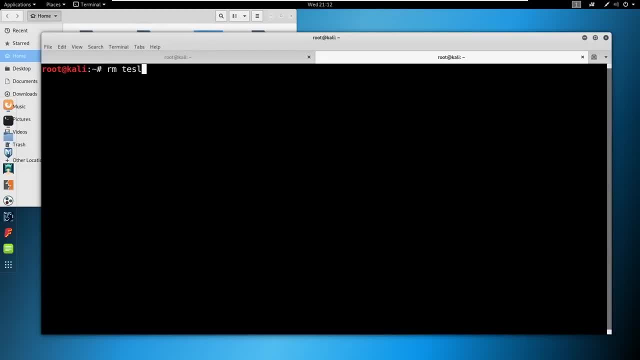 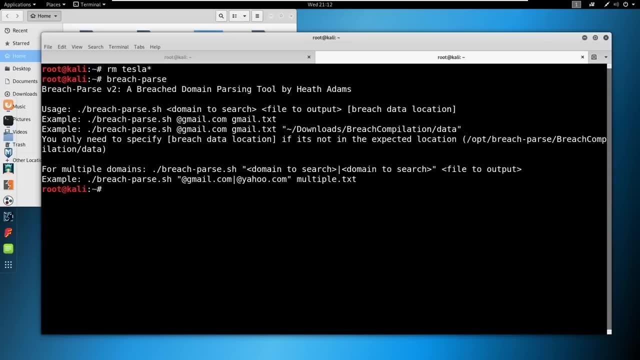 so i'm going to remove anything. tesla, that's already in here so we can run through it. i'll say breach, parse again. we'll get the- uh, the information from it. so i've got it hard coded already and i've got the files in the proper location. so all i'm going to say is: 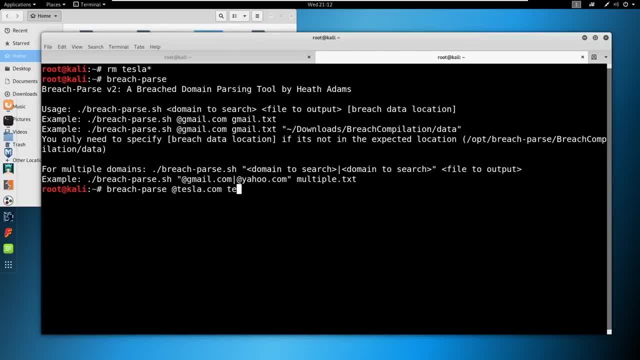 at tesla and i'm going to say breach parse and i'm going to say breach parse and i'm going to say teslacom and we'll just put it out to teslatxt and then that's going to run. so this will take a minute. while this is running, i'm going to go. 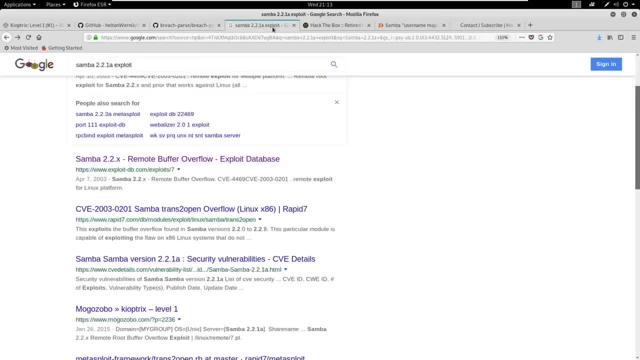 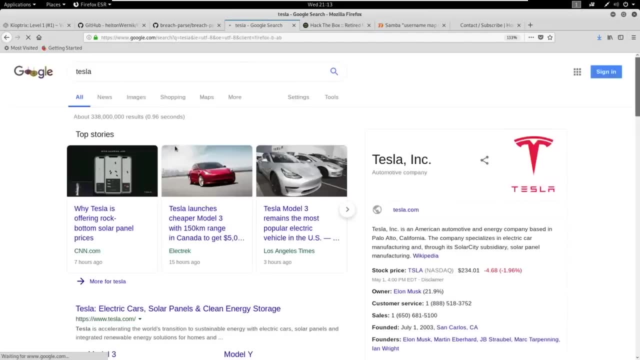 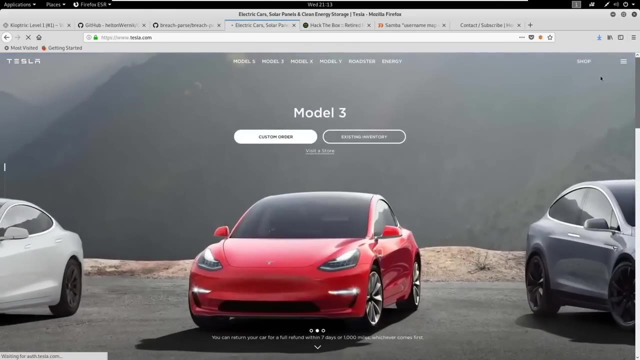 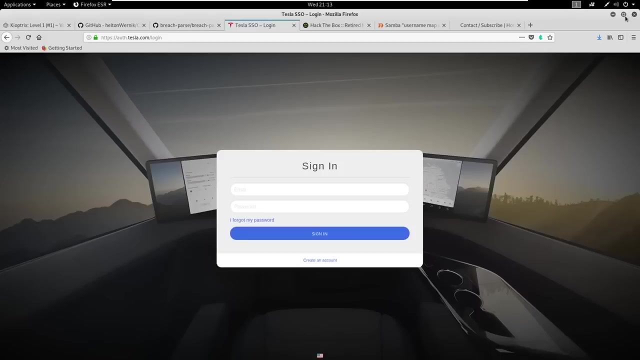 ahead and actually go out to the web and see if we can find some sort of login page for tesla. just for funsies, give you guys a burp suite lesson while we're at it. there's a sign in what do you know? all right, we'll do a burp sweep lesson, sweet lesson. 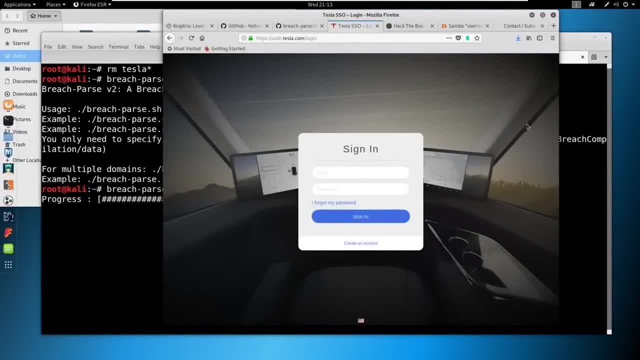 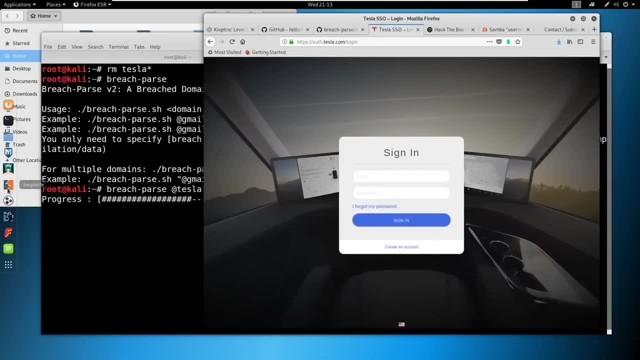 burp suite s-u-i-t-e. it's this fun little logo right here and i'm not on my hacking machine, so i don't have any of my cool tools. that's okay if you followed along previously. oh, that's a pain. oh, it worked okay. 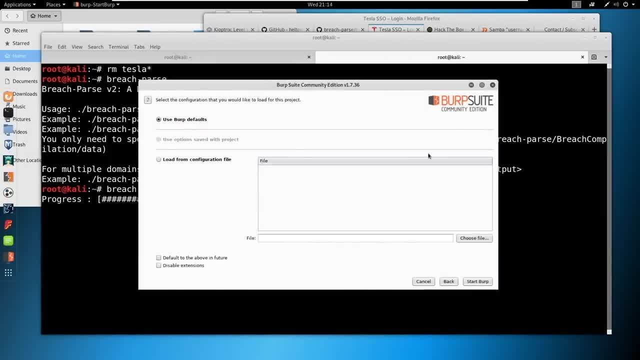 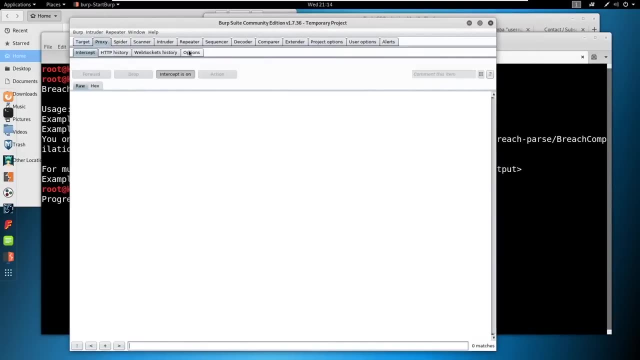 you followed along. previously i showed you how to set up foxy proxy, or told you to download foxy proxy at the very minimum. so be that guy who's got foxy proxy set up, but if you do not- and you're just now opening burp suite- 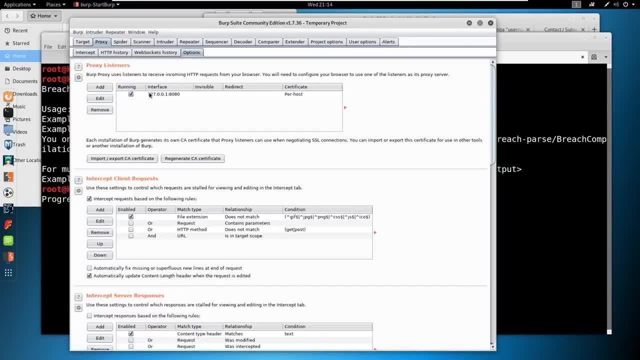 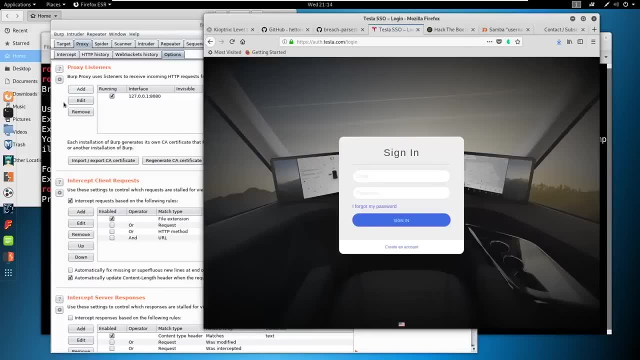 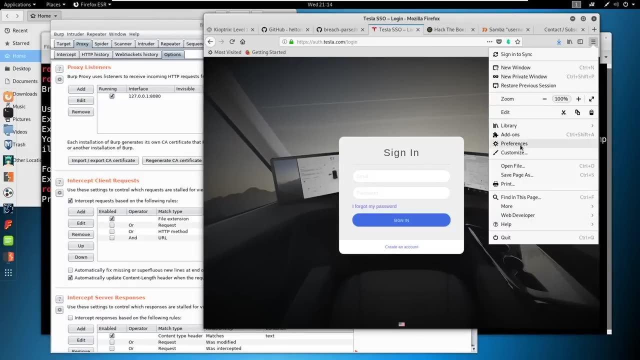 you come into your proxy and look at the options. we can change the name of the proxy. and we can change the name of the proxy. we can change our interface to this, the home address, with 8080. so i'm going to go into firefox, i'm going to go to the hamburger over here and do preferences. 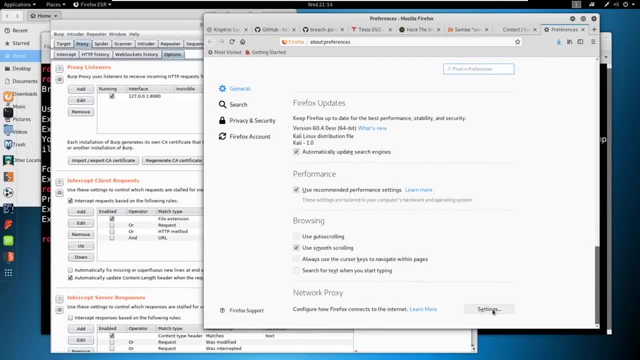 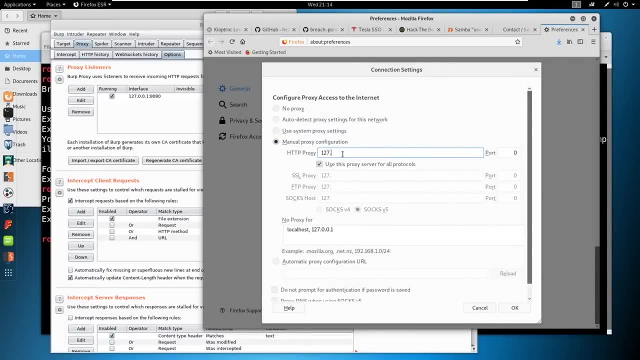 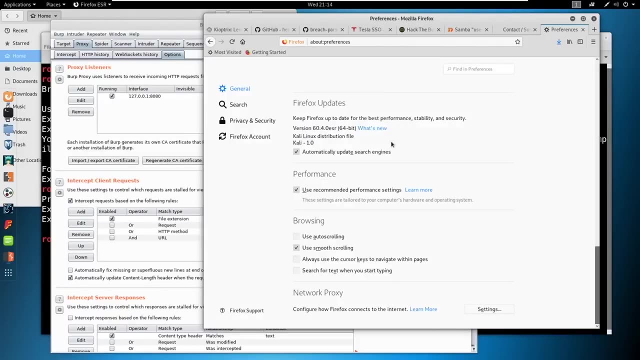 scroll all the way down. it says network proxy. you're going to click on settings, we're going to do a manual proxy, we're going to use it for all, and it's just one, two, seven, zero, zero, one, import 8080. okay, and then i'm just going to refresh this page. 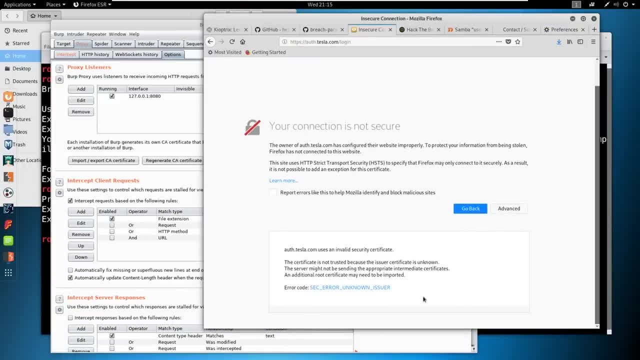 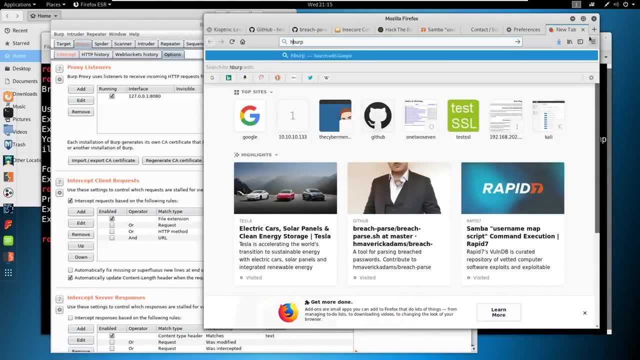 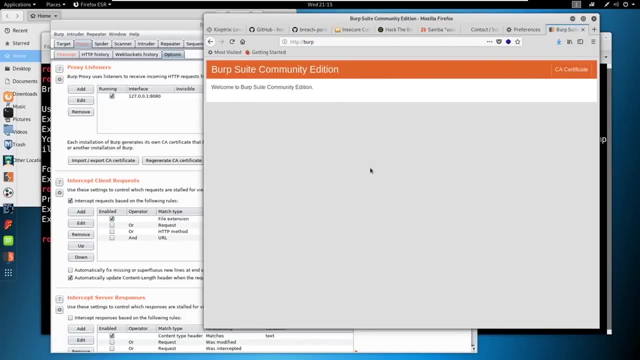 advanced. uh, i don't have the certificate either. okay, if you don't have the certificate, just type in burp, http, burp. if this doesn't work, i'll move over to the the other machine and we can run it from there. i'm just going to see where this came out. 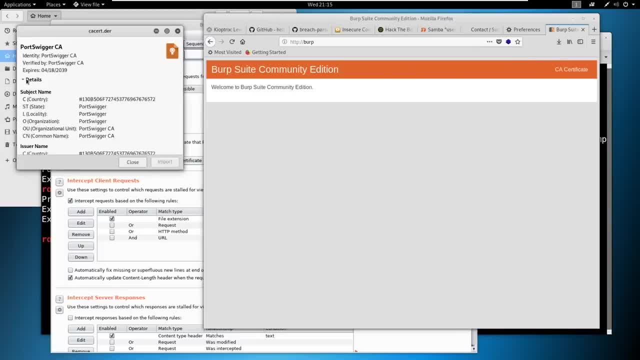 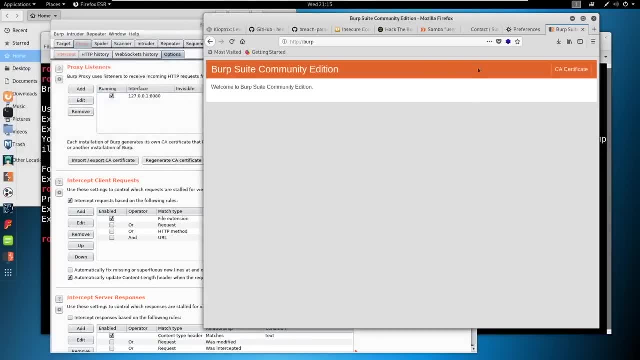 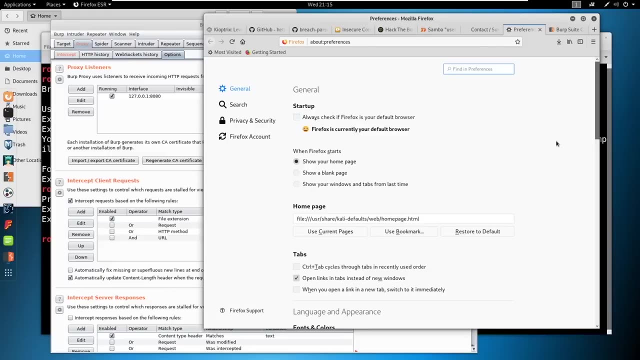 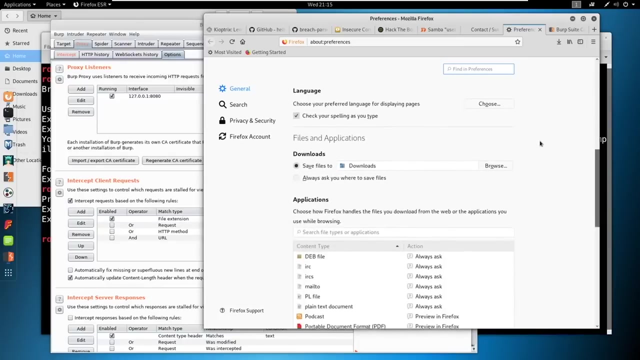 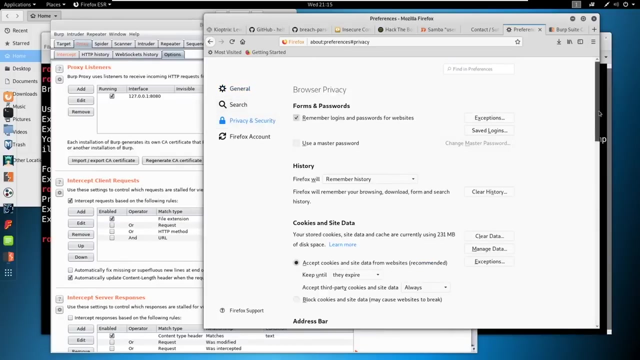 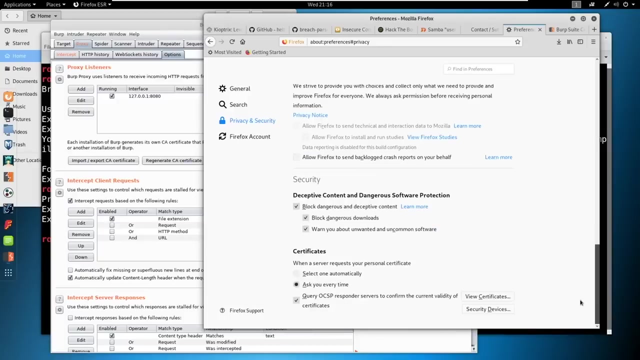 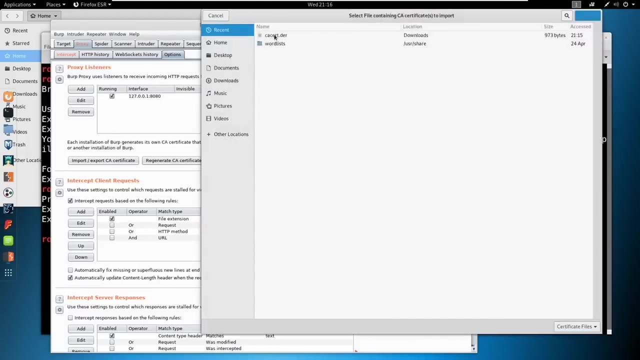 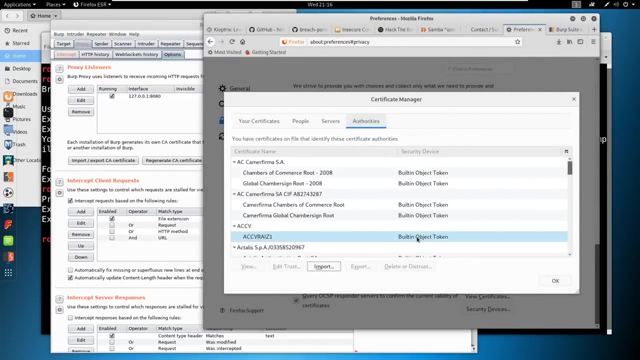 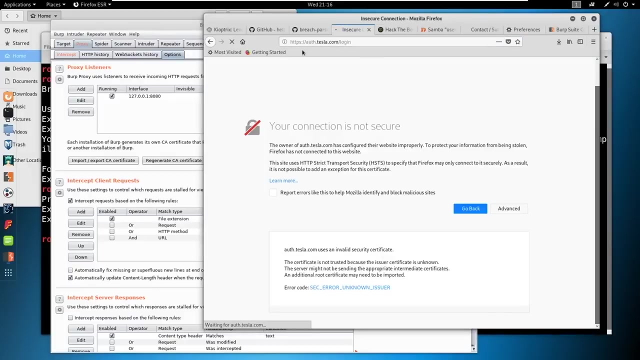 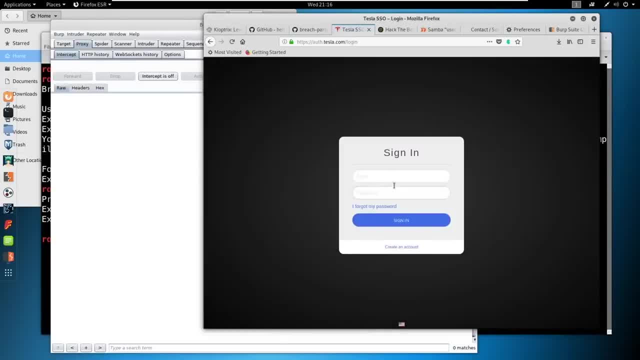 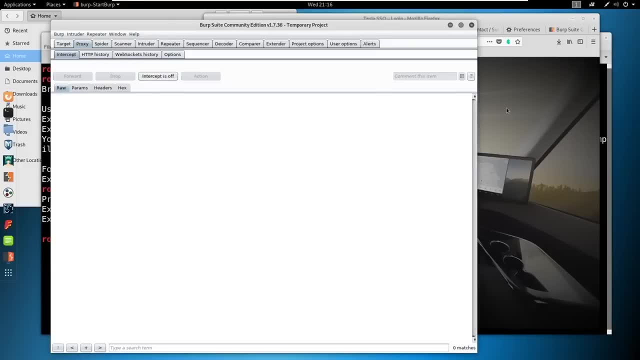 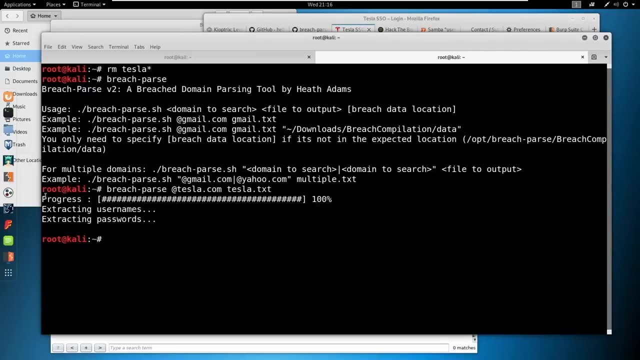 So it's working now. That's what we wanted. We wanted that intercept to hit. So again, if we refresh with intercept on, we want that to hit, We'll drop the intercept for now. Okay, So we've got our Tesla password list here. 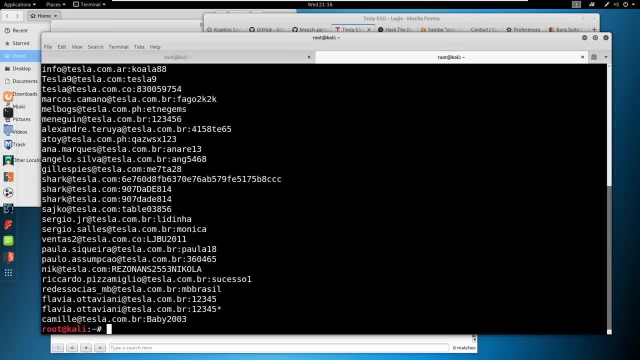 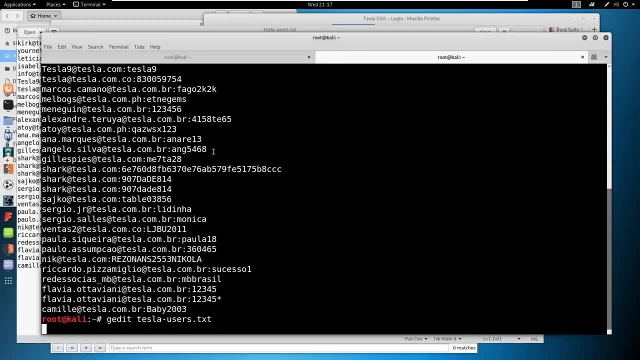 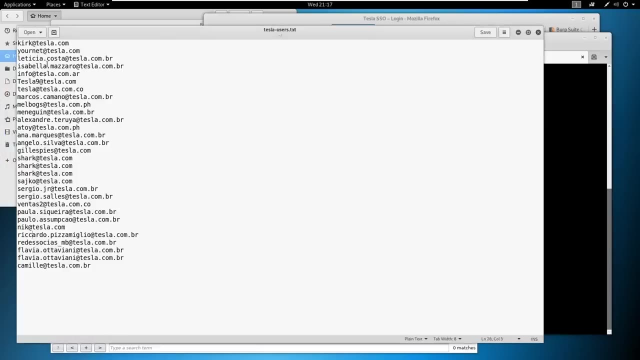 So if we cat Tesla Master, You can see we've got this Tesla list, I'm going to go ahead and just gedit Tesla users And you can see that it just split out the users just the way it was, And it's going to split out the passwords as well, in the order that they were found. 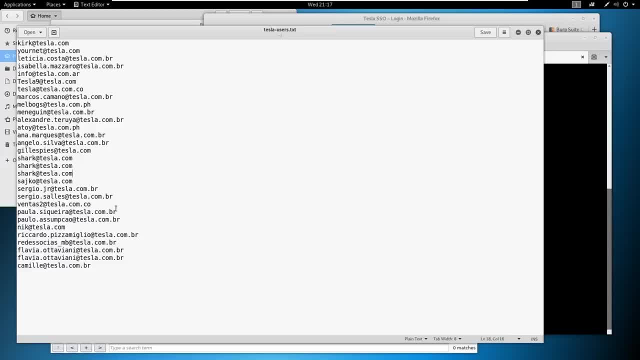 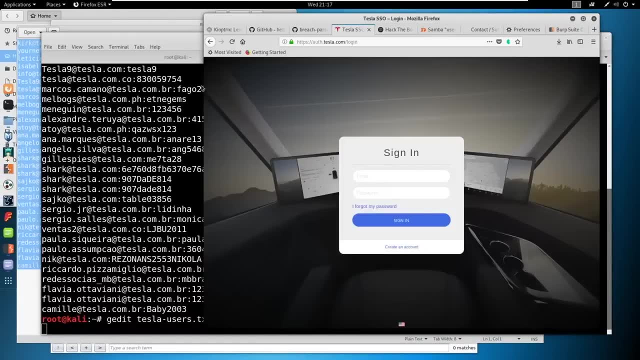 against the users. We're just doing an awk against it. Is this on the real Tesla site? Yes, it is. Teslacom is part of a bug bounty program. This is free game, So here's what we're going to do. 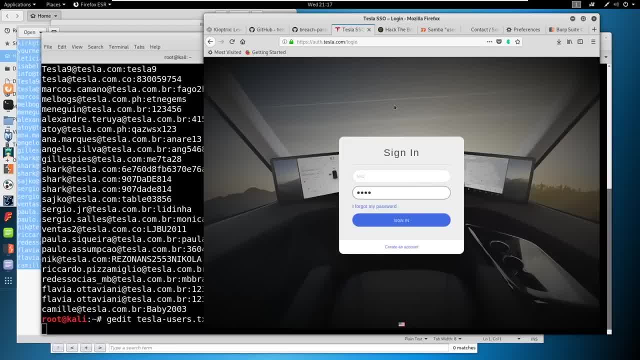 We're going to say: test for the email, test for the password, And you can see this is actually an SSO. It says Tesla SSO at the top. So we're going to go into burp and burp suite. free community edition sucks, but it is what. 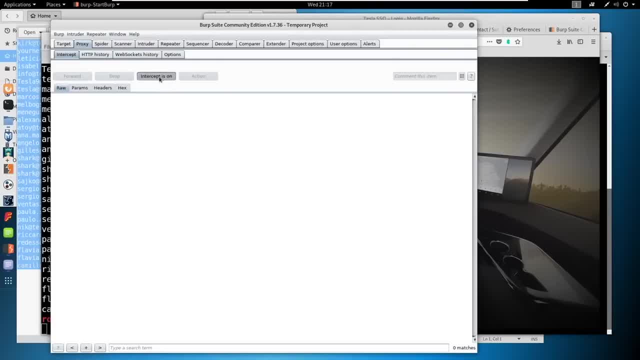 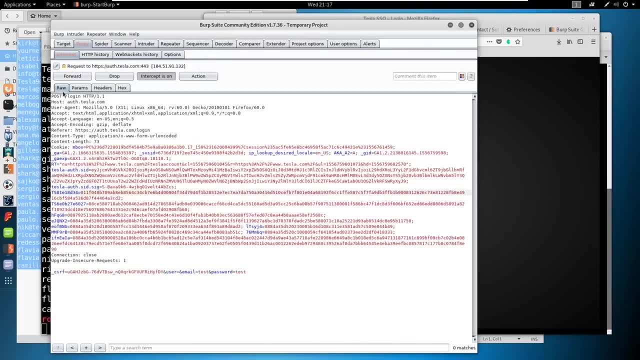 it is. You're just going to get to see what it looks like, All right, So we're going to say: sign in. We're going to intercept That request. Here's our request, right? We're sending this post request and it's got all the cookies. blah, blah, blah. CSRF token. 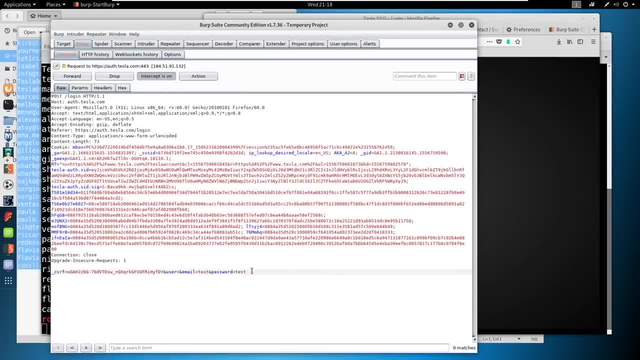 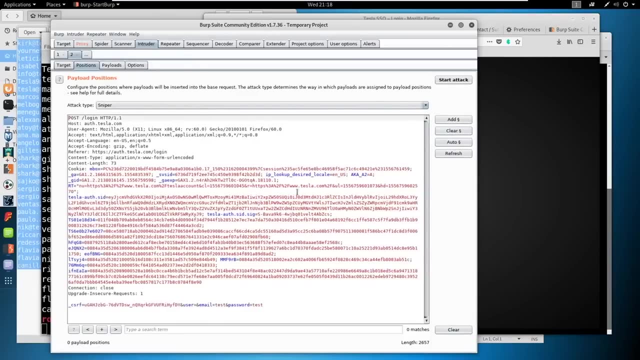 It's got the email and the password. burp pro is now $400.. Okay, We send this to the intruder, We're going to clear everything in here And then we are going to set Okay, So we set up our email. 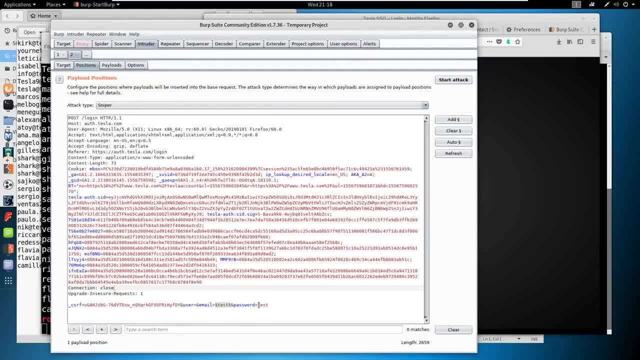 Tests. We're going to create a couple of positions. So we're going to highlight this test on the email, We're going to hit add. We're going to highlight the password, We're going to hit add. So now we've got one position, two positions. 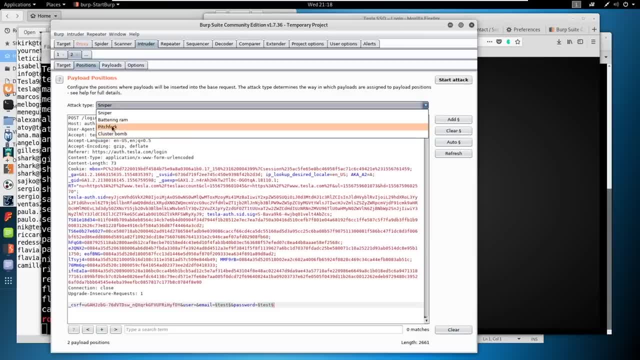 Now there's four different attack types for the specific attack that we're running. we're going to be running a pitchfork attack, So we come into payloads and we're going to say, okay, the first payload, payload set one. that is position one. 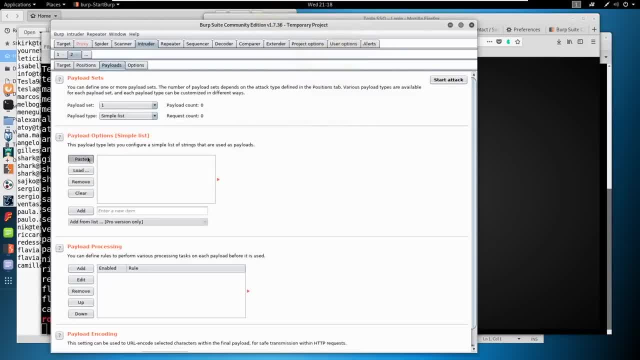 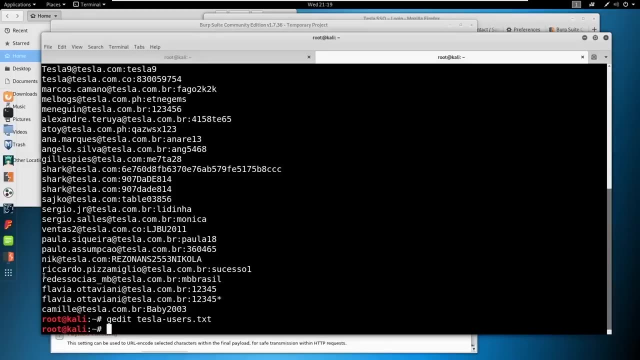 one that is your email address. we're just going to paste. we got all the emails in here, got 30 emails, right. we've got no requests yet because we haven't pasted a full request, because everything in payload set 2 is missing. so guess what we got to put in payload set 2: the passwords. so I'll just say passwords. 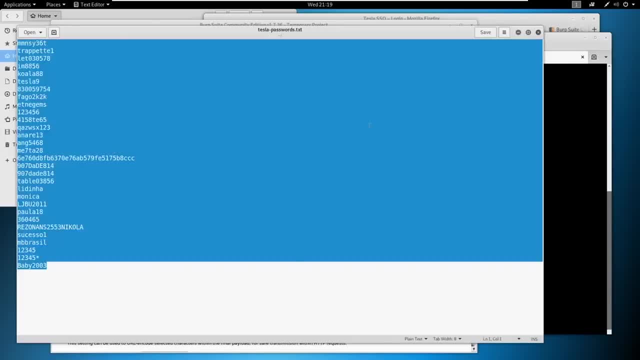 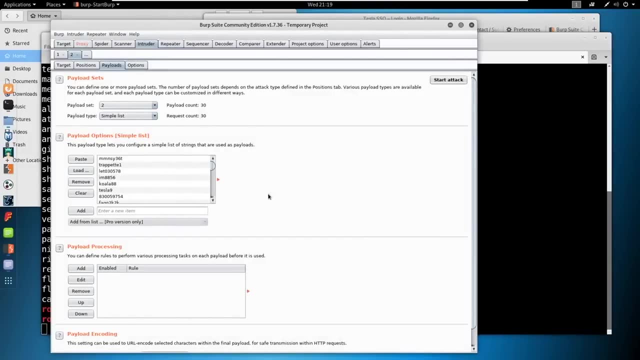 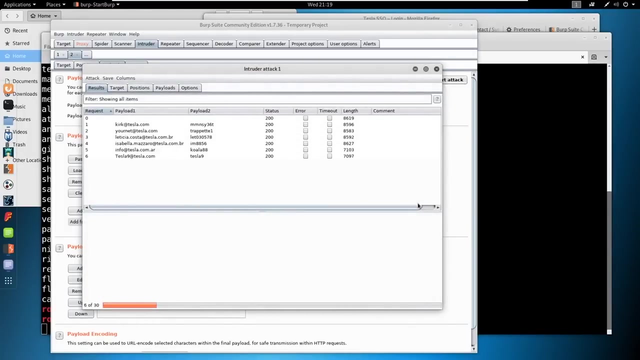 we'll copy all these and we will paste. now we've got a request of 30, we're gonna go ahead and fire this attack off. it's gonna say: burp intruder. some functionality is disabled. it sucks. okay. there are some things that we really, really need to be looking for here. you can see the length changes right, so 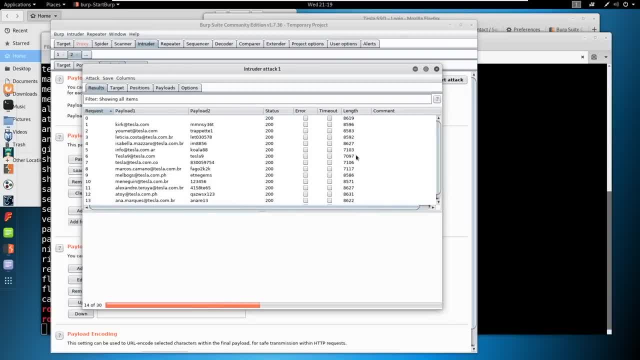 some things are really interesting. if we have a difference in length, that could be a really. it's an indicator that something is different. right from 8500 to 7100, that's a big difference. something might be there. you would want to look at the response that we sent. most of these are 8500- 8600, so I'm 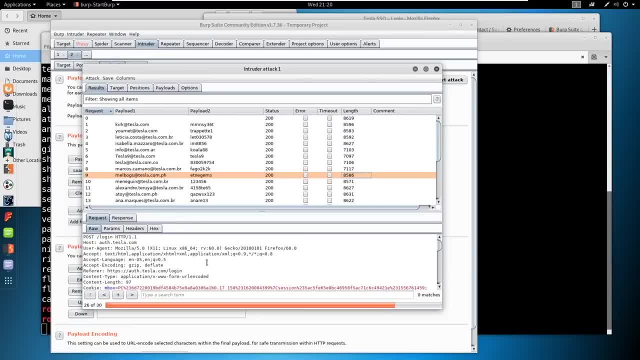 guessing that there is some sort of rejection, right, if we come into the response, we can even render it, and maybe it renders. we cannot sign in with the information you provided. well, that's good. they're not giving username enumeration, right, and we'll talk about that in a second. but let's look at the 7100 and see what that render looks like. 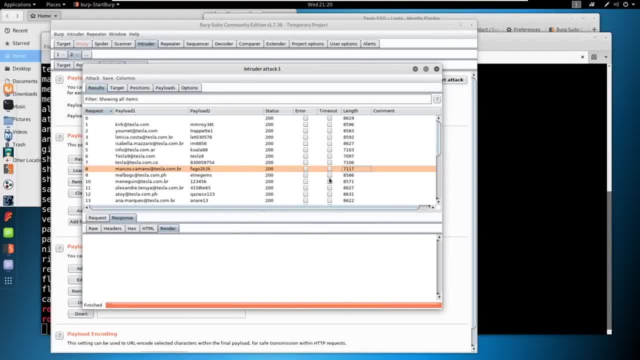 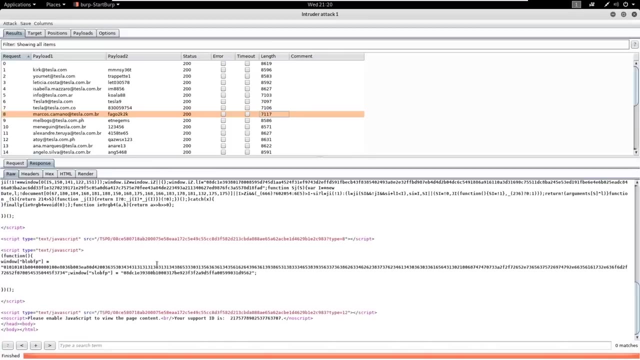 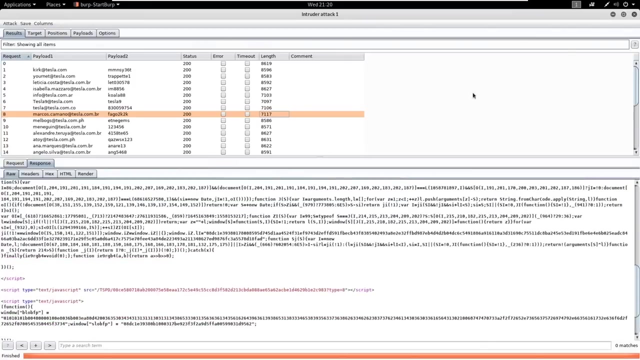 if this breaks in or something crazy dude I I'm done for the night, so I'm not trying to break into Tesla on a live stream. let's see what the the raw response looks like. please enable JavaScript to view the content. all right, let's try this user. 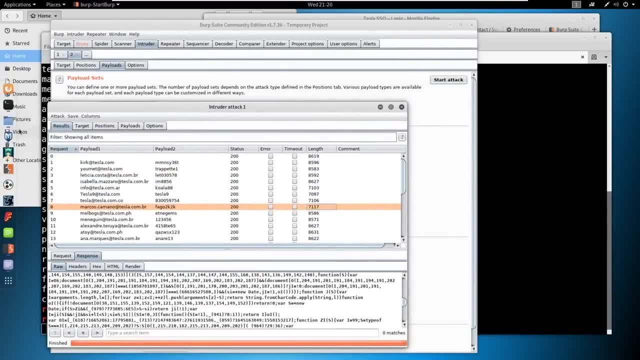 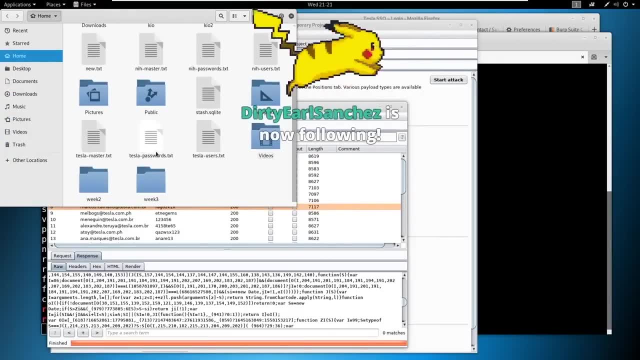 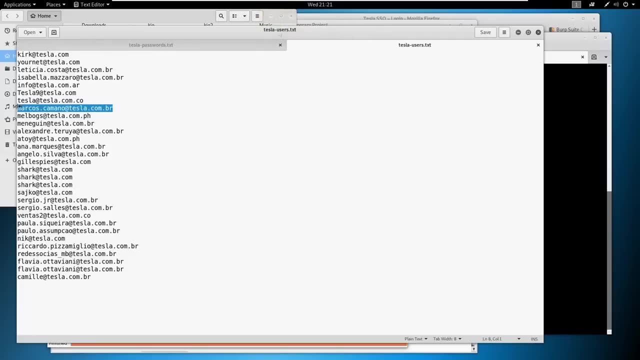 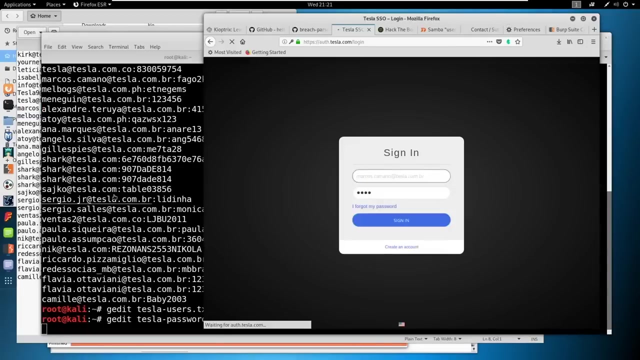 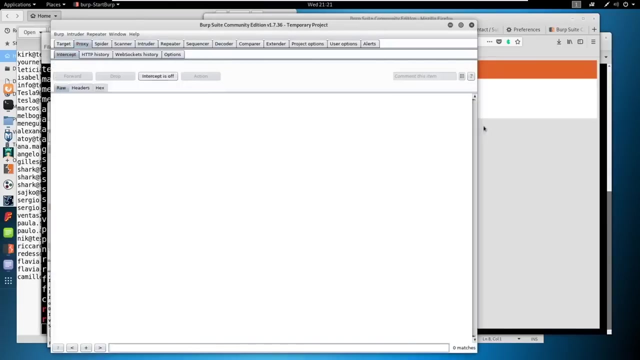 and password. fuck it. who is this? this is Marcos Camano. I'm sorry, buddy, if this is you, you, you, you, you. let's go to the login page. oh, we still got the burp intercepted. what we're gonna do is we're gonna drop that. okay, so we're gonna paste that back in and then 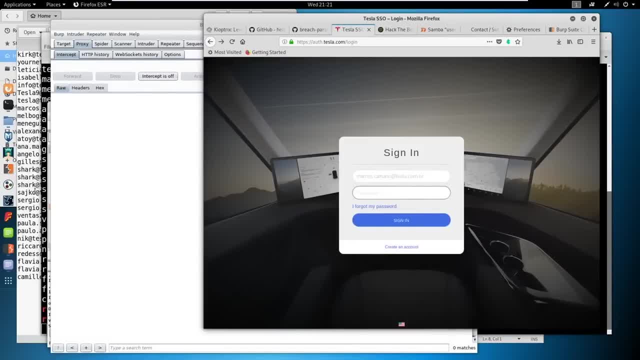 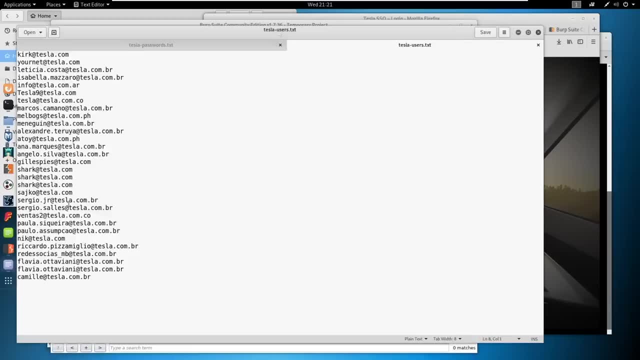 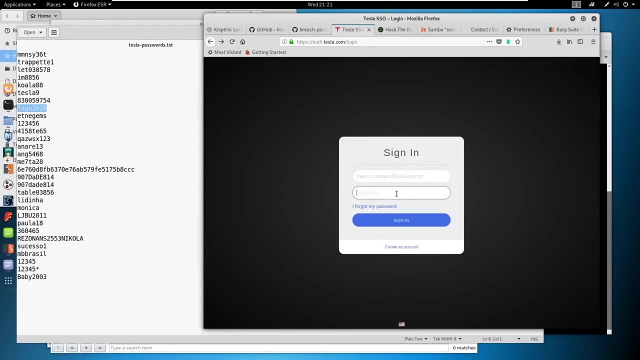 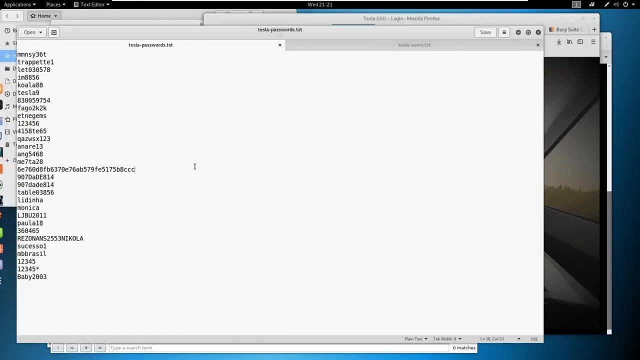 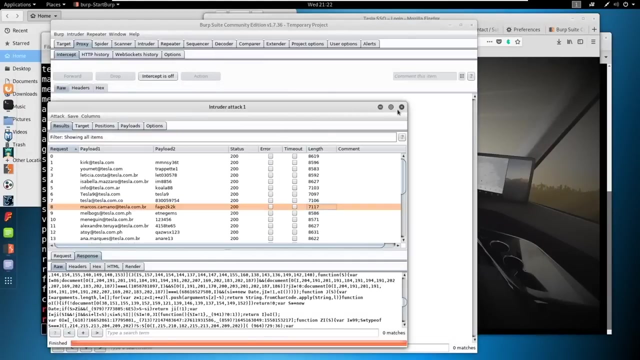 we're gonna say: find out what his password was. his passwords: Faygo 2k, 2k. okay, here he is, sign in. we cannot sign you it. so, for whatever reason, it was giving us a different response there for a second we can come back and look at this. I like. 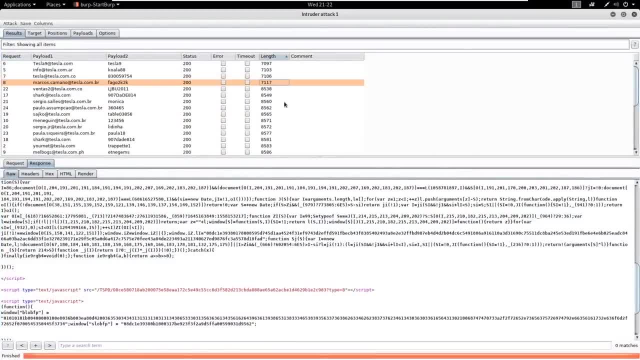 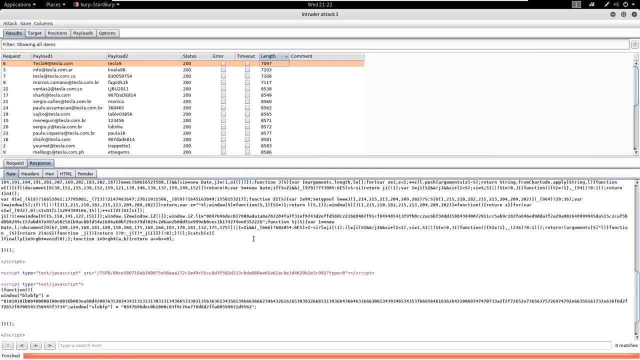 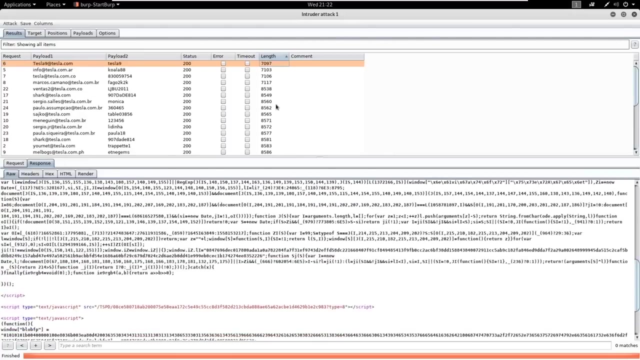 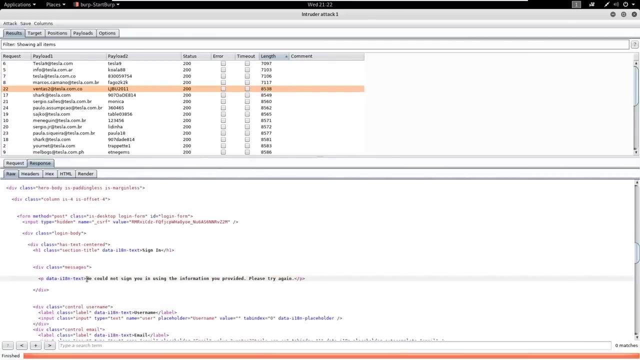 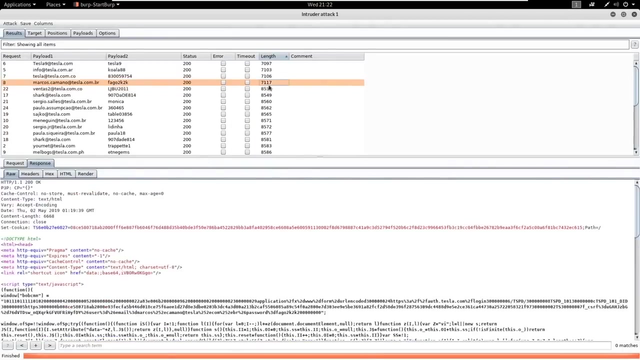 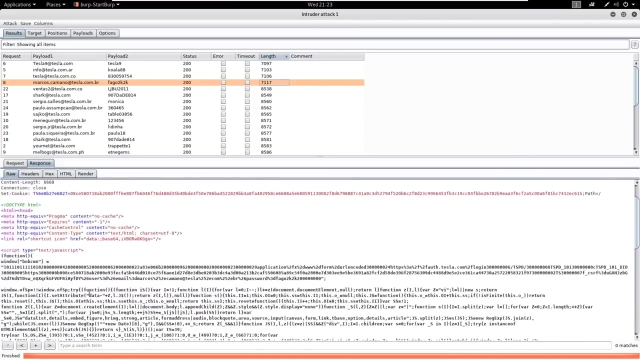 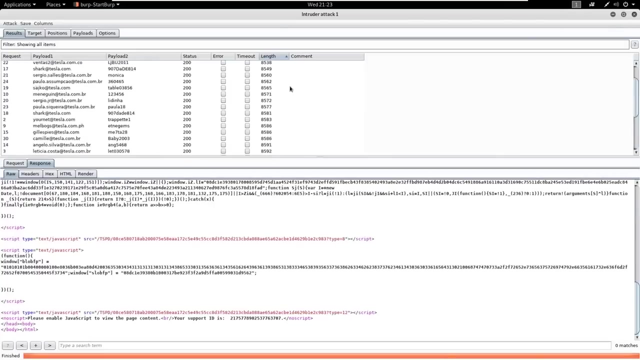 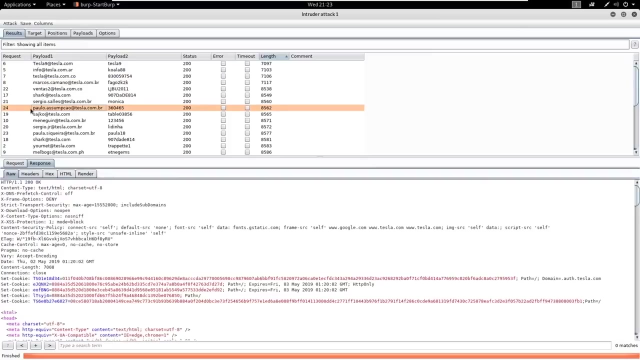 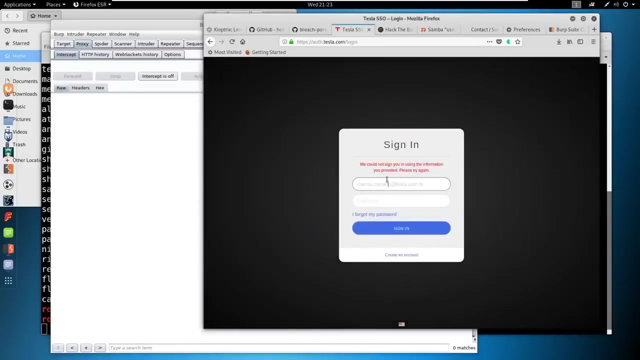 to sort this by length. you, you, you, you Broken The the background, Not off YouTube, if you were, or if you where everything as best as they possibly can, I'm not expecting much. They're saying we cannot sign you in with the username information or the information you provided. This is giving us no indication. if 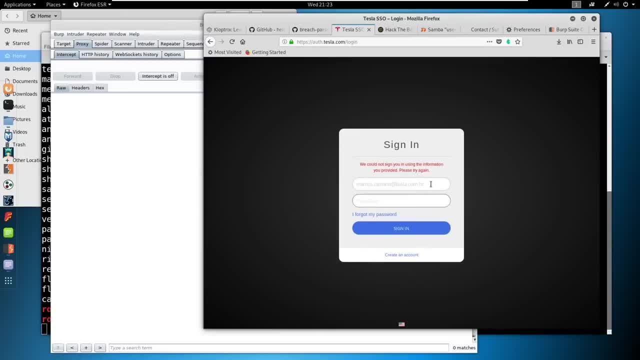 there is a valid user or not a valid user. Some websites will say: oh, you entered in the wrong password. Okay, well, that response tells me that the user is valid, but the password's wrong. Uh, in which case we need to change our, our type of attack, right, If we know the valid users? 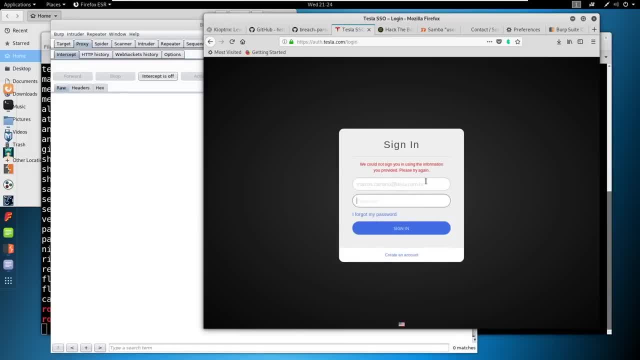 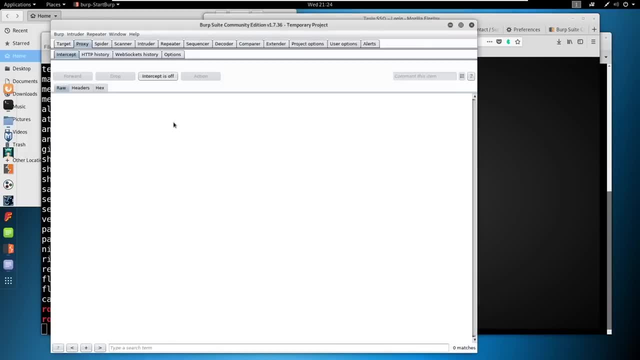 but we don't have a correct credential that we've pulled off a website. Now we can start our strategy and start doing something called password spraying. Spraying is exactly what it sounds like: you are spraying and you are praying. Now let's take a look at our intruder again. 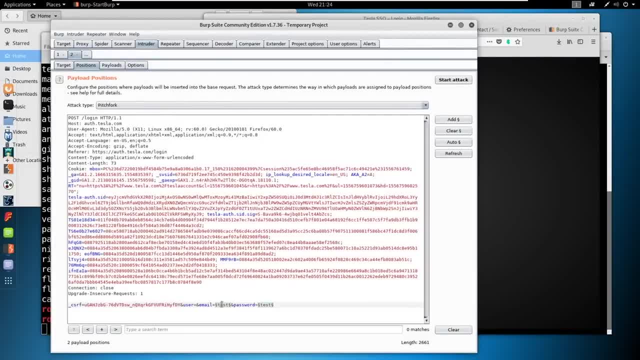 And let's talk about what we have. We've got an email set and we've got a password set. but what if we clear this? Let's go back to the email and we'll put it as test And for a password, we'll change this. 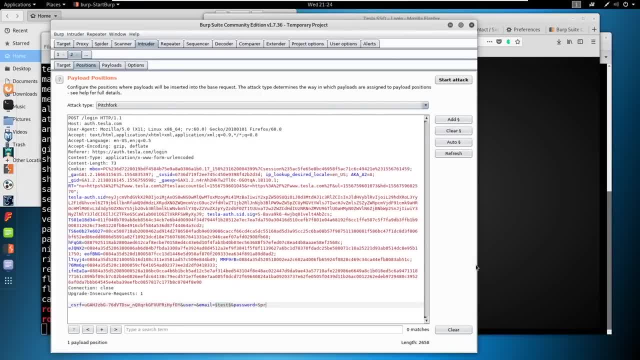 We'll say: what is it right now? Is it spring, Technically, spring 2019 exclamation- That's a really common one, Or you do the the the season before winter 2019 exclamation, or password one. or Tesla one, two, three. You just start making up passwords and seeing what sticks. 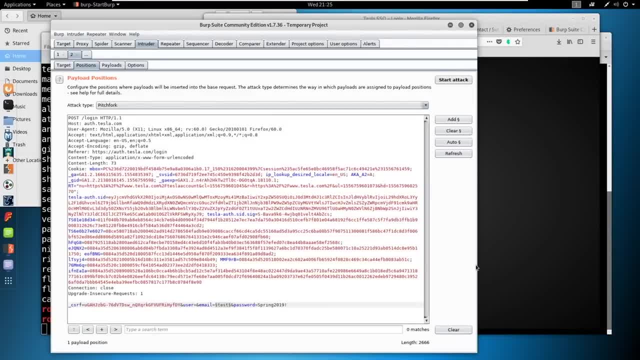 This works out really well. So let's go back to the email and we'll put it as test. Really really well, If there are no protections and sort of like a limitation, a user lockout, et cetera, If they're just letting you fire, free game all day. 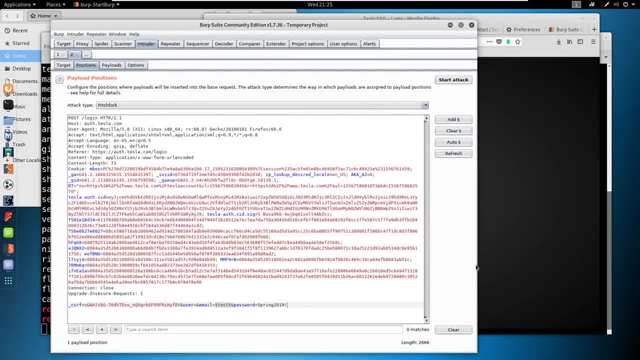 it's only a matter of time before you get a good, valid password, So we'll hold constant at spring 2019.. Now we could set this and come up with a list of like 10 or 15 passwords and let them fire off as well, But for just this example, we'll just set. 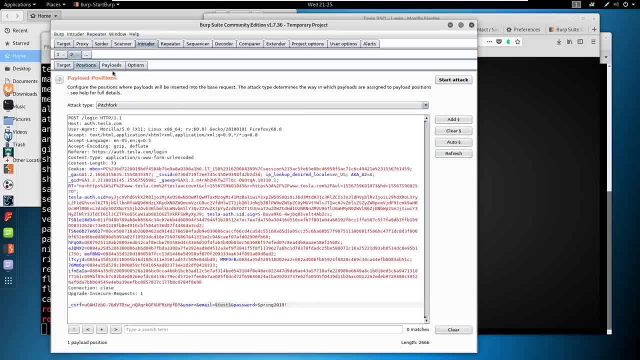 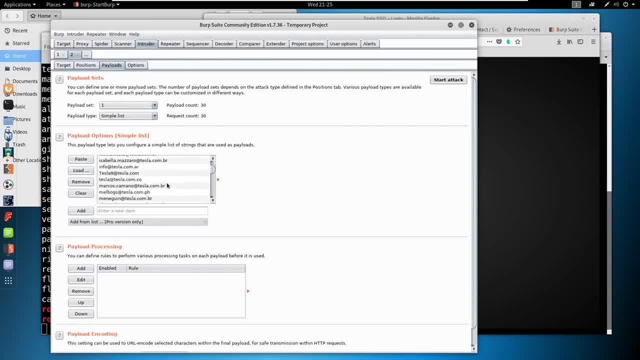 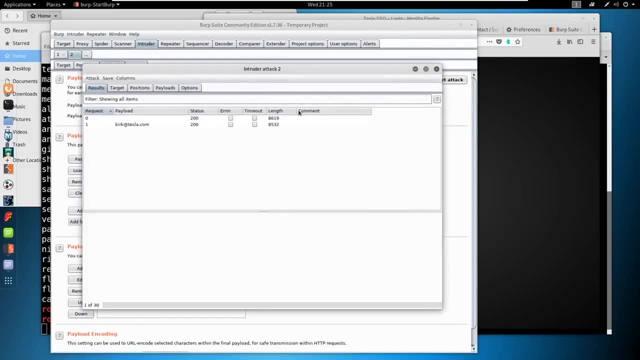 this. We'll hold constant to spring 2019 and we can come into the payload. And now we've got one payload. This is called a sniper attack And what we'll do is we'll have all the emails coming through and we'll just snipe it off. So it's going to send- uh, Kirk, you know your net. 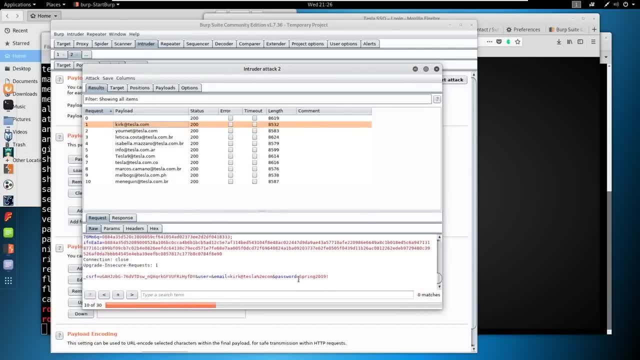 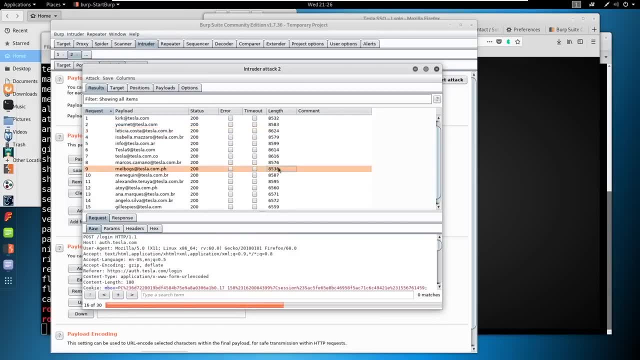 whatever It's going to send that request with the password. We've told it the spring 2019.. You can see kirk at teslacom. Uh, it'll send it all through Just like that. Now there's a bunch of 8,500 and then one came down again, the dot BR, So maybe. 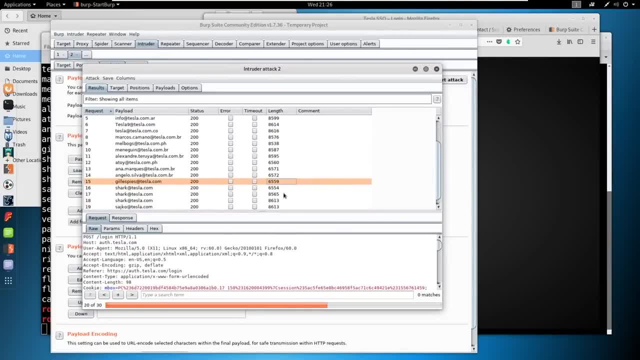 the BR, is it? but it looks like a period of time where it's actually limiting us. If you see the requests in a row, we got 1110 in, actually the zero, no 11 in, and then it starts going into 6,500 and maybe blocking our requests. I think it is actually responding, Vita. I think it is. 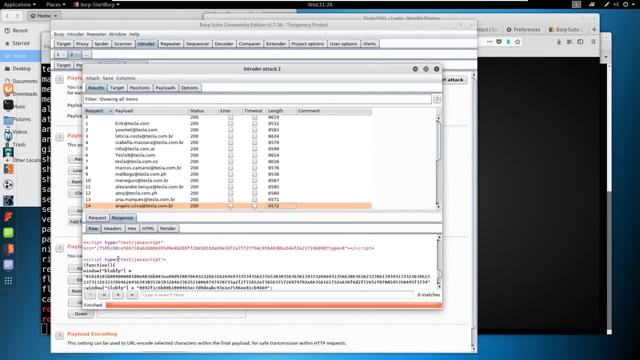 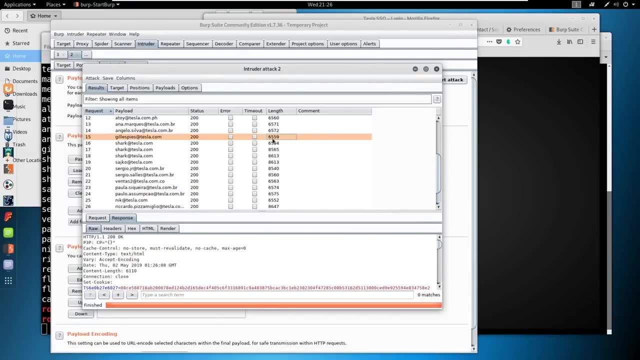 responding. I think that's what this is. Um, if we're being honest, I think we sent too many and it's it's blocking now our requests here and then it comes back through, So it kicks us for a minute, but this is the concept of 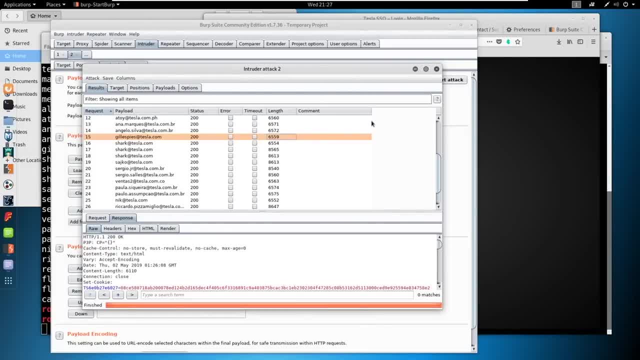 password spraying. So if you go and watch uh that that talk I was talking about. uh. this is one of the concepts that was used to actually uh get into uh a VPN. So credential stuffing doesn't always work, uh, but you can use it in. 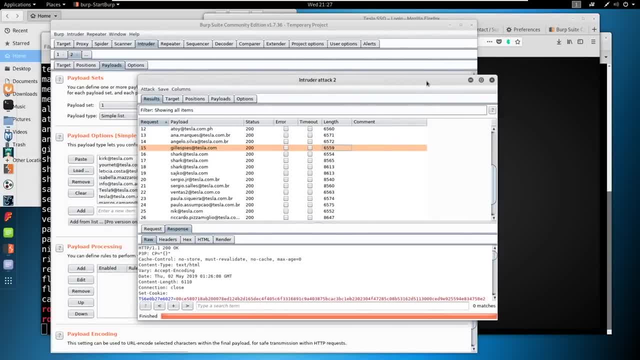 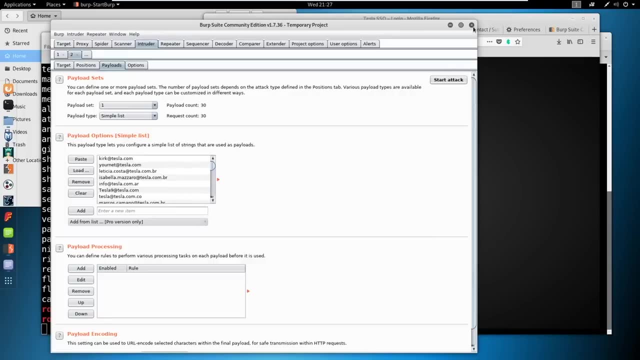 combination with password spraying And as much information as you can gather is a great way to get into a network when there was no other way previously. So we are at nine 27.. That is pretty much it for this lesson. I wanted it to go nine 30. I will call that an achievement, So I'm going. 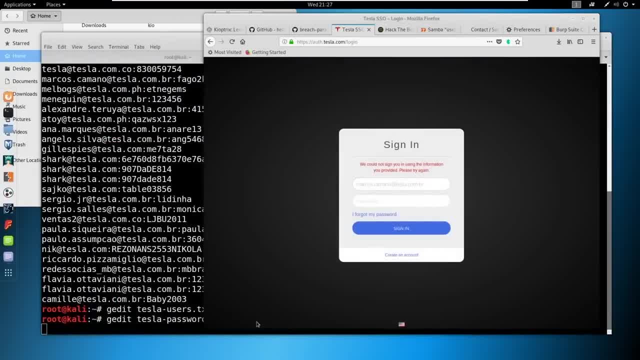 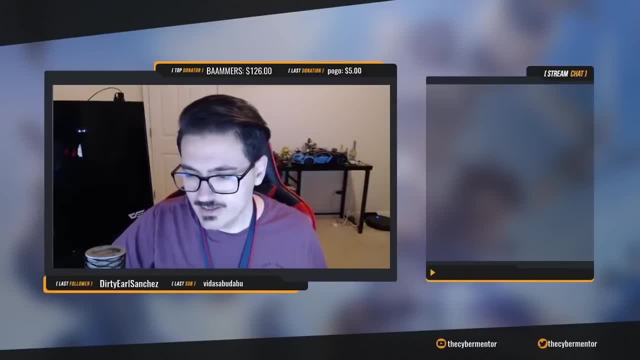 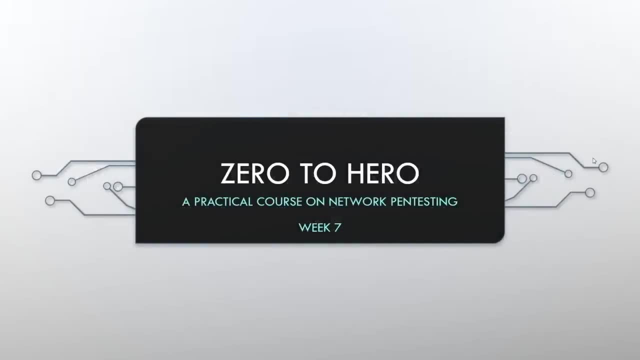 to go ahead and close all this And I'm going to bring my happy face back over. We will start our AMA Q and a. whatever questions you may have, It is not week seven is week eight. You can tell that I definitely didn't put a lot of effort into 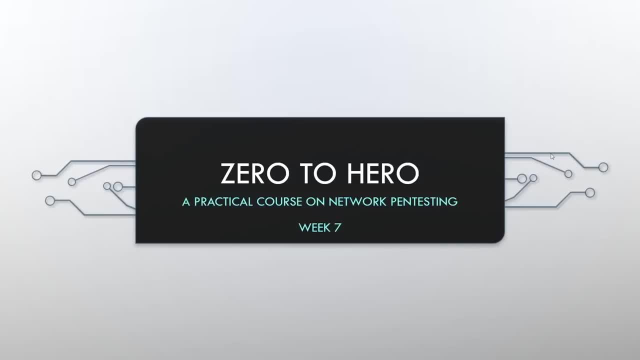 this PowerPoint. As you'll see, there's only three or four slides. Welcome to week eight of zero hero, So today's video is going to be a little bit different. I'm going to go ahead and show you what I'm going to be doing, So I'm going to go ahead and show you what I'm going to be doing, So. 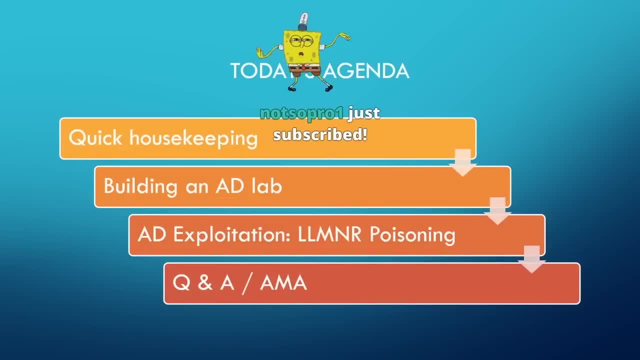 I'm going to go ahead and show you what I'm going to be doing. So today's agenda got a little bit of uh, of housekeeping, very, very quick housekeeping. We're going to build an active directory lab. We're going to do a little bit of AD exploitation tonight and then we're going to do our AMA, like 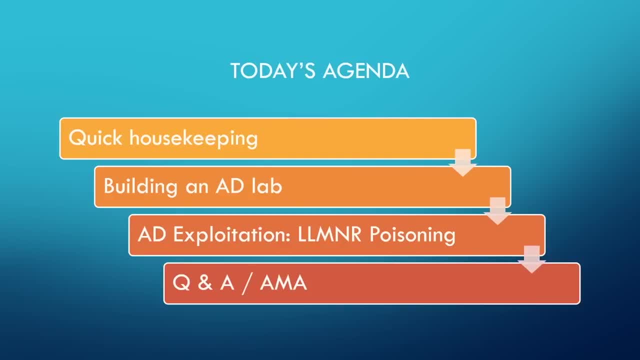 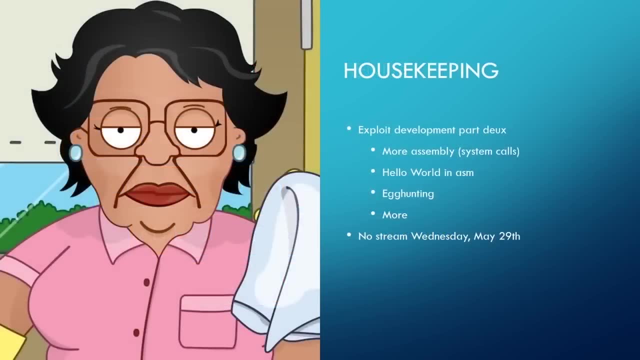 always. Thank you, Not so pro for the sub. I appreciate that. All right, Housekeeping. tomorrow night, eight o'clock Eastern, That's the same time This is starting. your favorite person, Joe, will be back. Rory will be back. He will be teaching us exploit development part two. 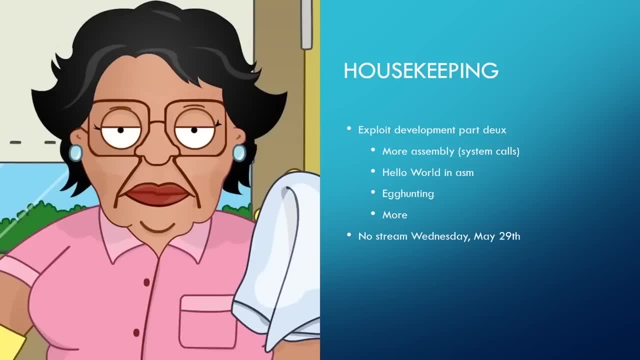 So we're going to be doing more assembly, focusing on system calls. He's going to be doing hello world and ASM. He's going to be doing some egg hunting and a little bit more. So if you are behind on the series for exploit development, go to the YouTube channel and check that out. 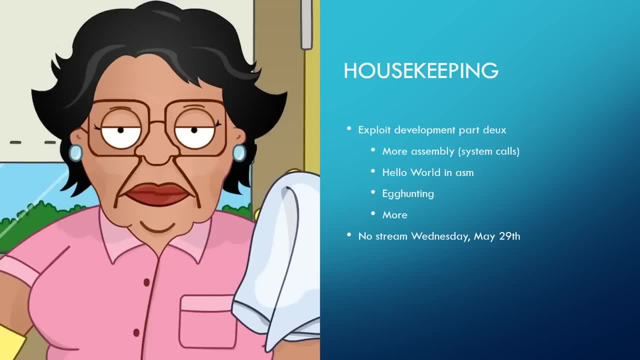 Do some catch up before tomorrow night. It should be a good stream. you guys liked him last time a lot and he wanted to come back and you guys wanted him back, So Joe will be here. Other news- And I am going to repeat this on every stream leading up, because 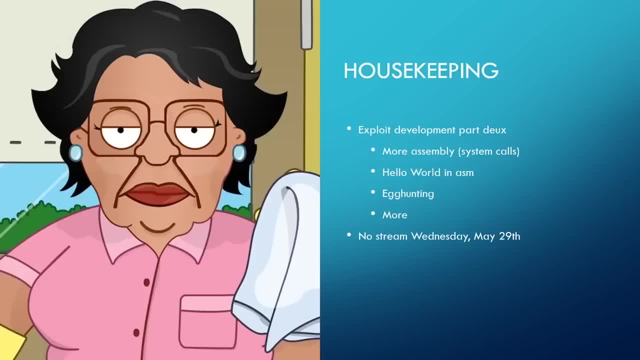 you people will forget no stream on Wednesday, May 29th. So the goal right now is to have this course finished, maybe by the end of this month. I haven't figured it out. We're going to spend three weeks on active directory, I think maybe two weeks. 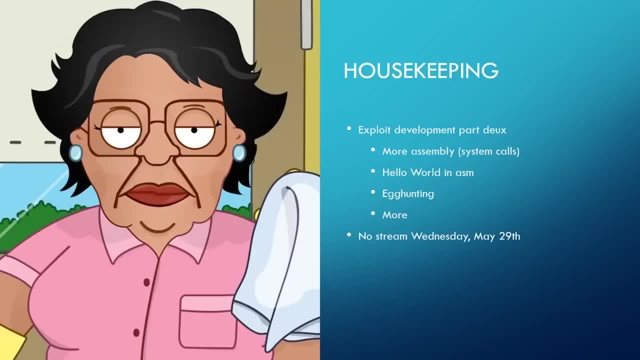 And what we're going to do is: on Wednesday, the 29th, I'm going to be out of town, So we may do a double stream Monday and Tuesday of that week and wrap up the course That way. we can. we can knock. 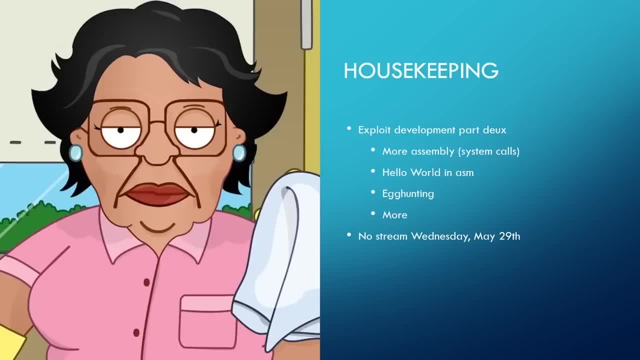 it out by the end of May, And then June we'll start fresh with something new. I don't have everything planned out yet, But but hopefully we can get it all done. We can say we went zero to hero and wrap up this course. So that's the goal for now. That may change, but do not forget to 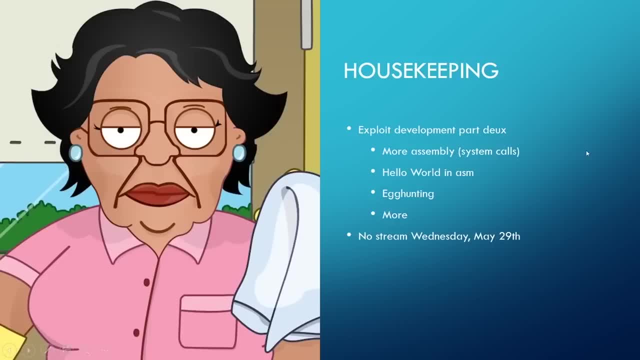 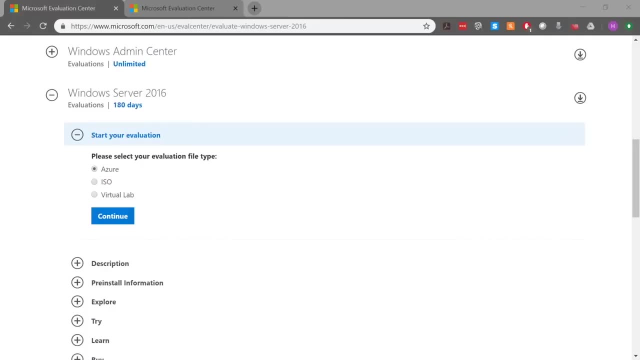 subscribe to our channel And we'll see you next time. Bye Again. no stream: Wednesday, May 29.. We don't need this slide yet. That is for later, All right, So I sent out homework to you guys. The homework was to just download a couple of ISOs. ISO number one: 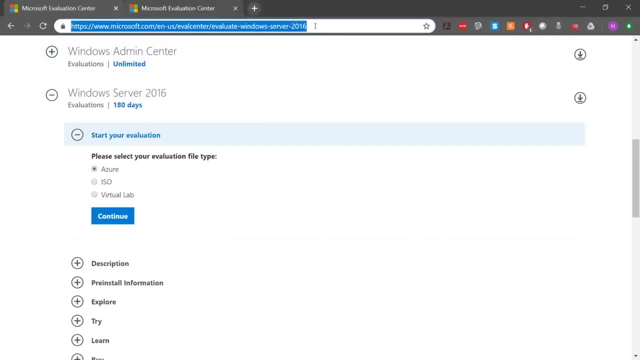 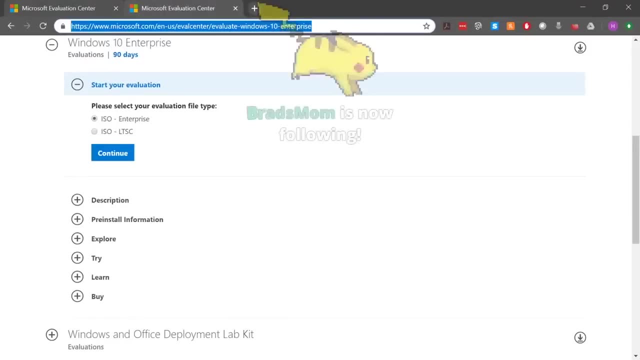 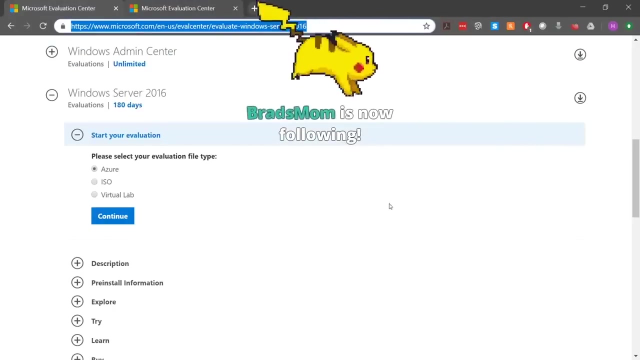 is this: Windows Server 2016.. I'm going to copy this and paste this in the chat if you don't already have it, If you're not on the mailing list. Also, Windows 10 Enterprise, And all you need to do is if you're watching this at a later time on a recorded video. 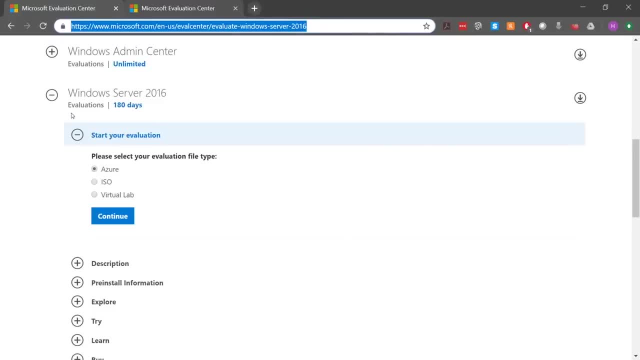 come into this area here for Windows Server 2016.. It's an evaluation of 180 days. That's perfect for our lab. Just click ISO, hit continue And then you enter in some information: first name, last name, company name, etc. Hit continue. They may or may not send you an email, really doesn't matter. 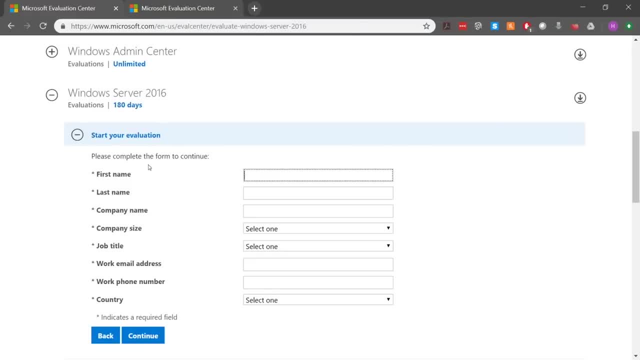 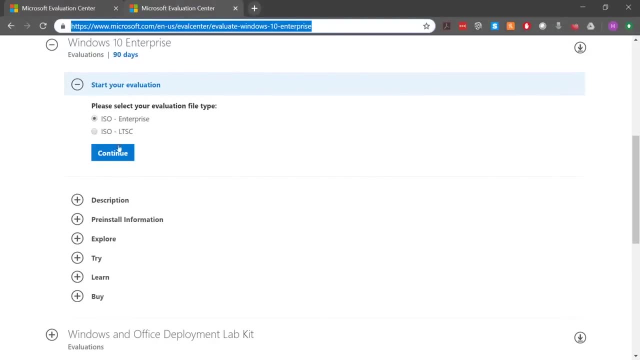 It'll automatically download the ISO So you can put in fake information if you'd like. Same thing goes for the Windows 10 Enterprise. you're going to say ISO Enterprise. you're going to hit continue on that and download it. So in a perfect world where we already have sent out the homework, we're going to say that that's. 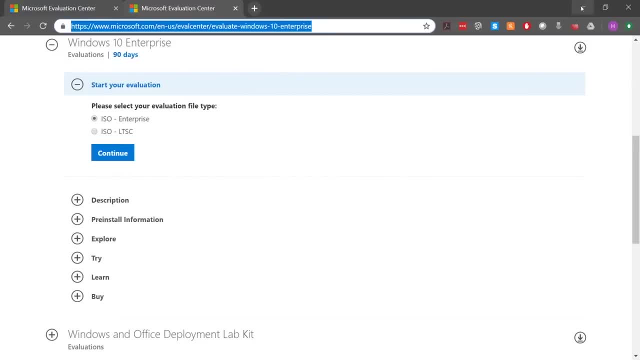 already done And we're going to just get started right away into installing these ISOs. Now, I could have had you install these yourselves, But there's a few- I'd say two, actually- quirks about this that we need to note in order to get it installed. 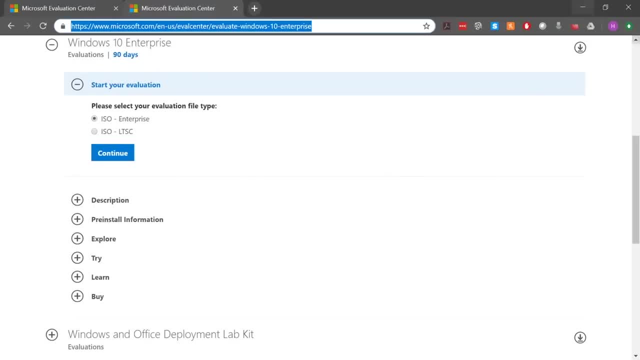 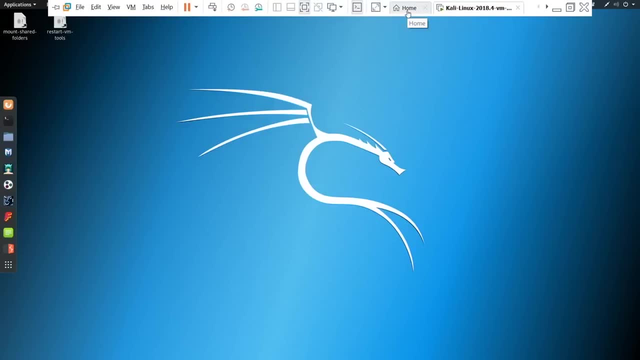 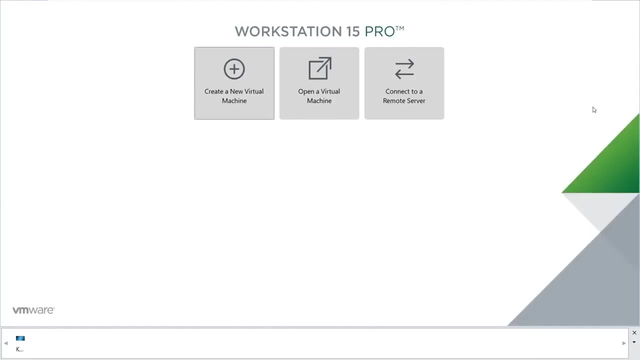 So let's go ahead and just take a look at that Now. tonight I'm going to be using my VMware Pro And I'm going to say a couple of caveats about what we're getting into in this course. That is that everything we're doing, we're gonna be running three VMs at once. If you do not have 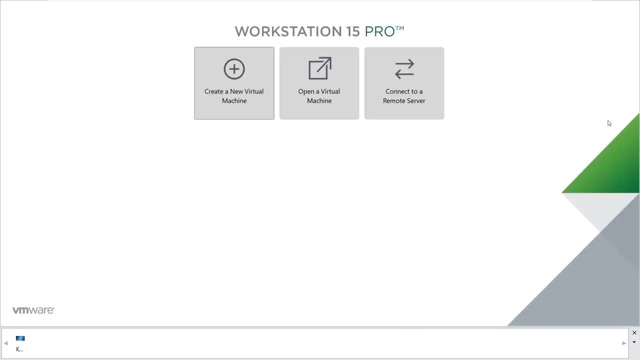 a lot of RAM or you don't have a super fast computer, this is going to be very slow for you, So make sure that you keep the settings at two gigabytes of RAM and just let things run. It's even a little slow for me because I don't want to stream, run three VMs and keep my fingers. 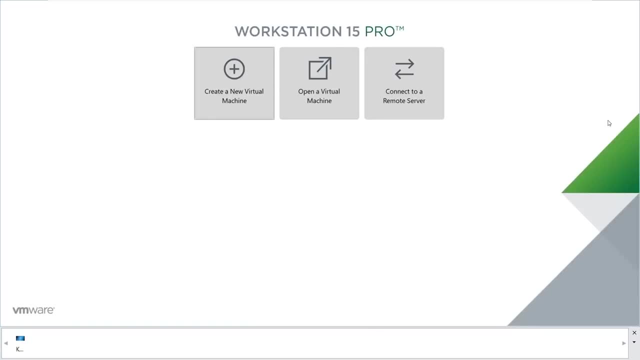 crossed. that's going to work or not. So we're going to build this out together. It may be hard to follow along if you don't have a super fast computer, If you don't just watch the stream. sit back, enjoy yourself and learn. you know, learn some lessons on how you would set up Active Directory. 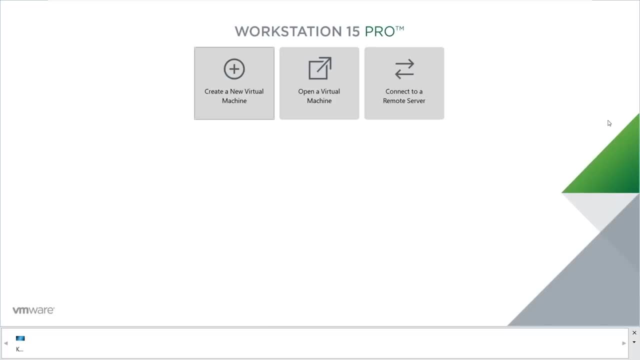 And we're going to cover the first part of the exploitation tonight with the LLMNR poisoning. So, sitting in Workstation 15 Pro, I'm going to hit create new machine. If you have just the regular workstation, that the workstation player, you're just going to have to. 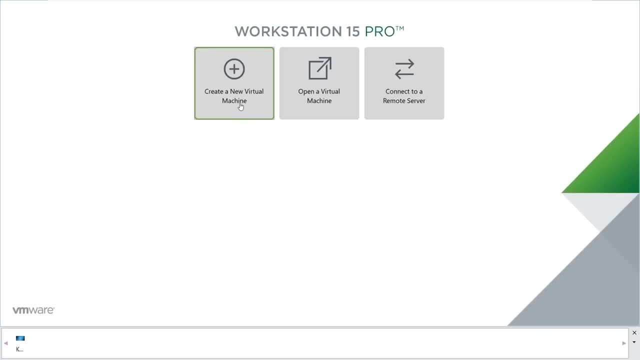 create a new machine, open another workstation player, create a new machine again and have all three running. If you've been doing that already with the previous lessons when we did cap tricks, you should kind of have a little bit of a hint on how to do this. So we'll create the new machine. 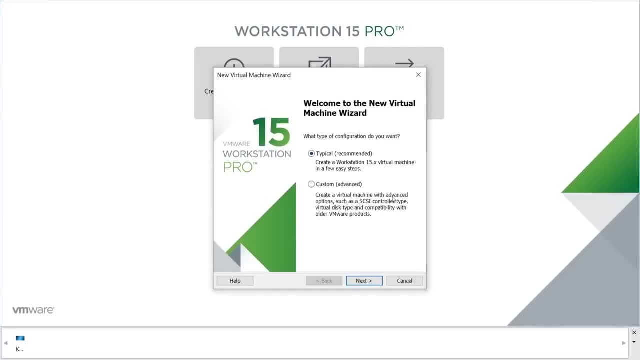 And it's going to say: what kind of configuration do you want? And we're going to say: typical. And then I've already installed this once before. So it's going to say: hey, where do we want to grab that ISO? I'm grabbing the data center ISO first. So we're going to install server 2016 first. 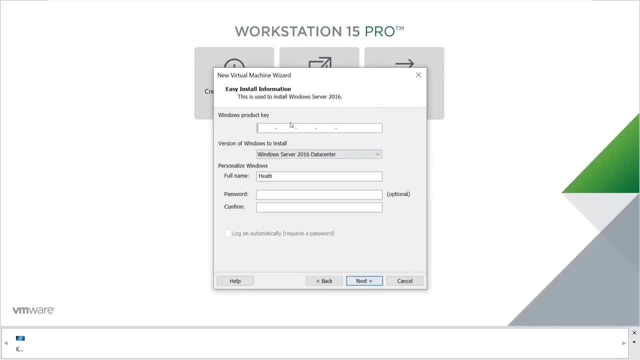 And we're going to hit next. Now it's going to ask you for a product key. We're not going to put one in because this is a test ISO, So we're going to say: Windows Server 2016 Standard Core. You can have your name- You don't have to put a password in here- And just hit next. 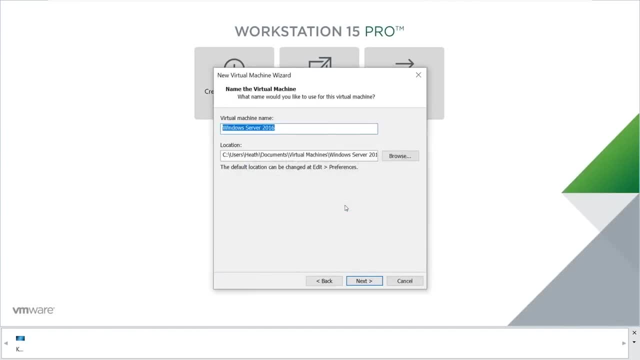 It's going to say you didn't enter a product key. Yes, we want to continue. Okay, it's going to try to put it in my users documents, virtual machines, If you've got space. I don't have a ton of space on my SSD, So I've got some other SSDs that I'm going to put this on to. So I've already made a little directory for it. I'm just going to copy and paste. Put this under Win Server, Hit next Okay, maximum size: 60 gigabytes is what I'm selecting. You could select less, I just leave. 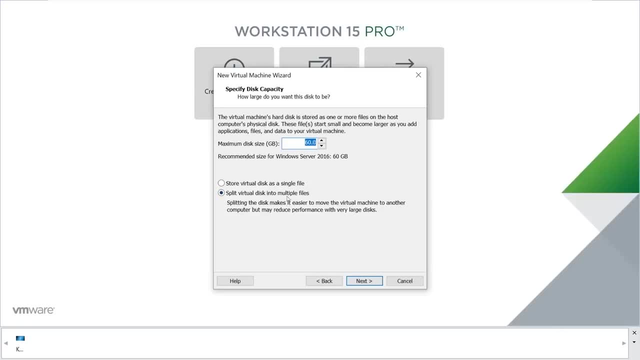 it at default, Because what we're going to do is we're going to do something called splitting the virtual disk, meaning that we're only going to take up the amount of space that we need, up into 60 gigabytes. You could also store it as a single file, and that will take up the full 60 gigabytes. 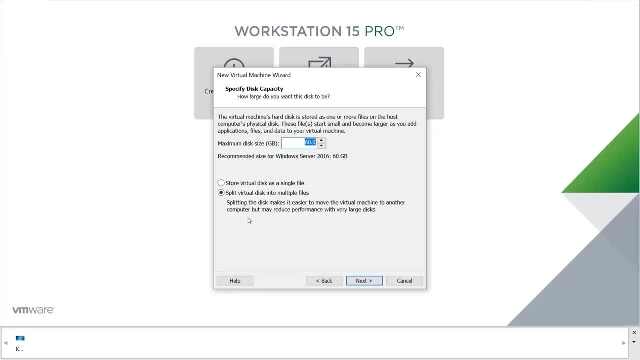 But this allows for expansion and doesn't doesn't take up the full size, I believe. So what we're going to do is just hit next on this And then we are going to make sure- by default, I believe- power on this virtual machine is checked. 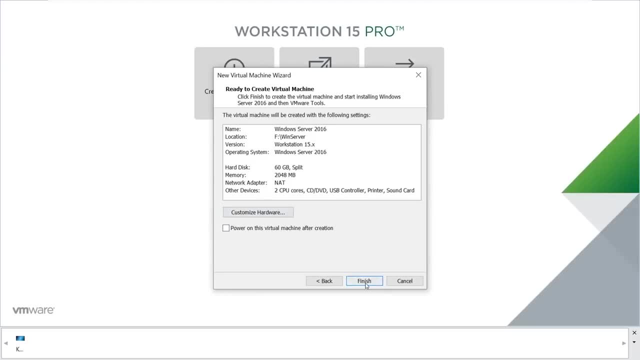 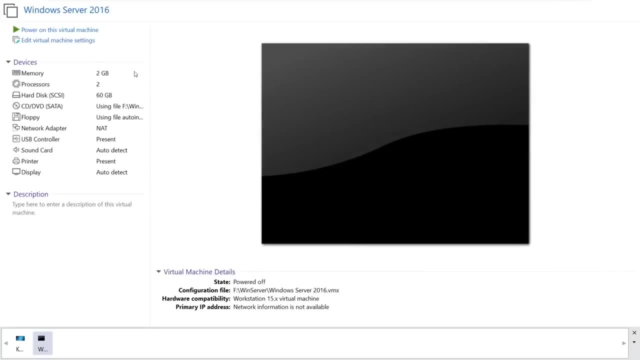 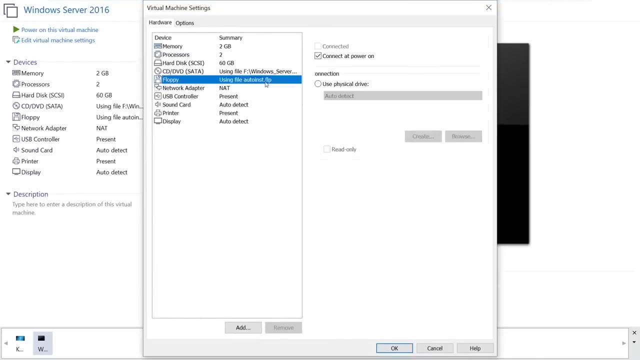 make sure it is unchecked And hit finish. All right. so now at this screen: Windows Server 2016,. let's go ahead and just hit edit virtual machine settings. What happens is they use this auto install floppy file for whatever reason, So it's got this floppy. 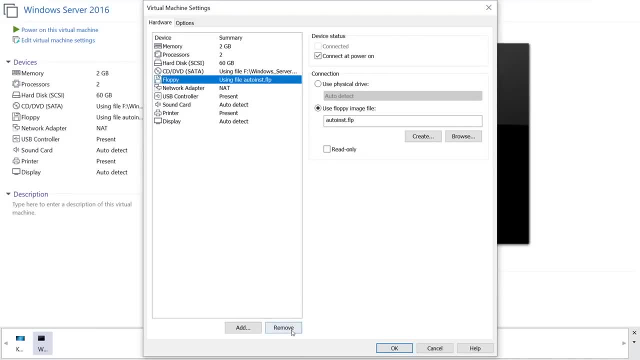 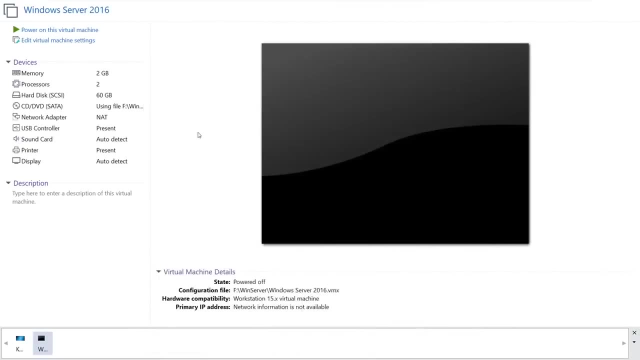 device here using this auto install. We're going to remove that because that causes a lot of issues on install. It's looking for a license and we don't have a license because we're just demoing this out. So let's go ahead and remove that and then we'll hit power on this machine and get your. 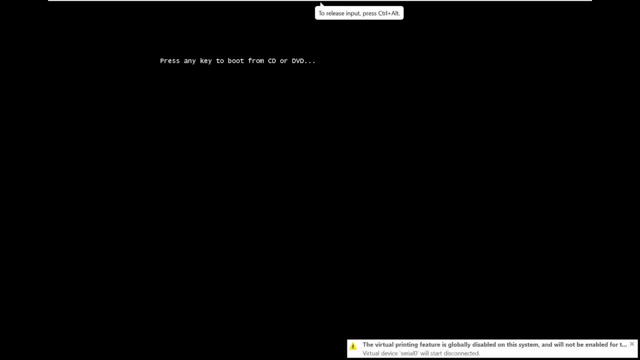 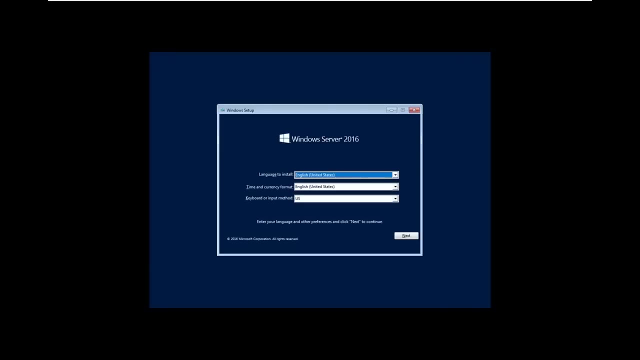 fingers ready because you're going to have to hit a key to continue Or else it'll go through the boot menu. try to pixie boot. I don't know why. that's the default boot method, So make sure that you are booting into this first. So if you've ever installed Windows before, this is probably boring. 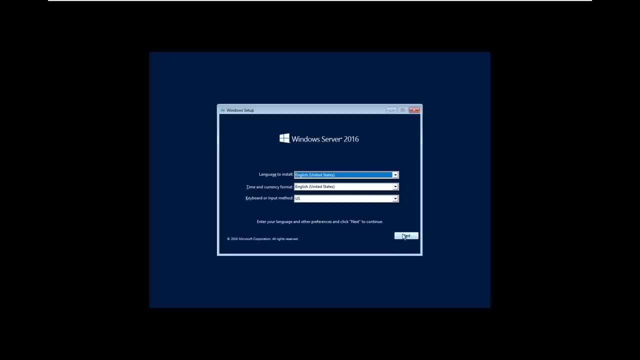 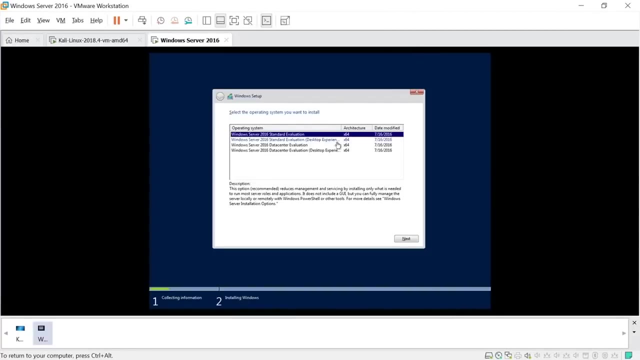 for you. I apologize in advance. We're going to hit next and hit install now And we'll let this run. Okay, we'll do a little bit of multitasking And I'm going to come out of full screen here. Actually, let this go into standard. 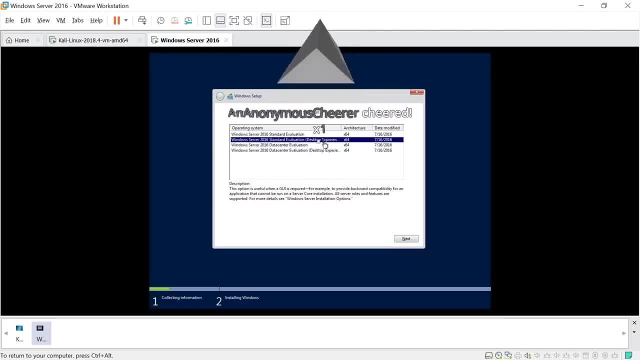 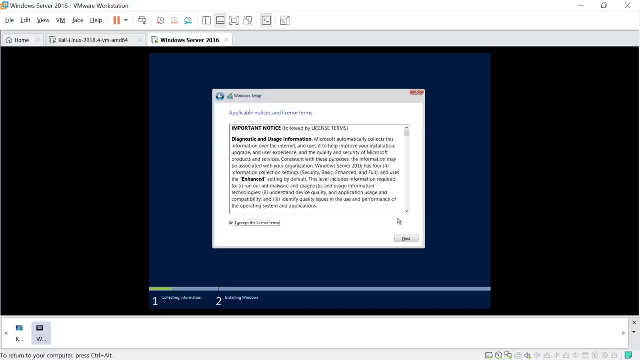 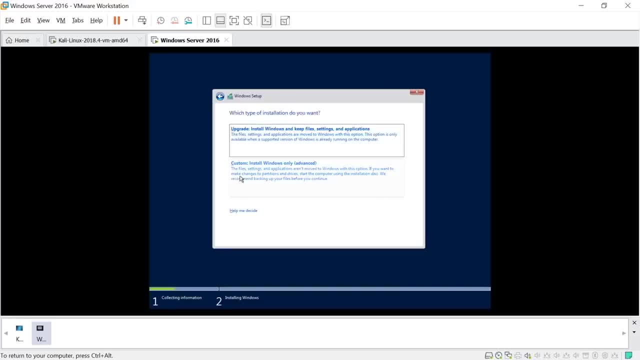 whatever it is that we do, We're going to select custom install Windows only advanced. We're going to hit this little new button down here. It's going to auto partition for us. Just hit apply. Say okay, Thanks for the sub FlutSec. I appreciate that And we're going to hit next. 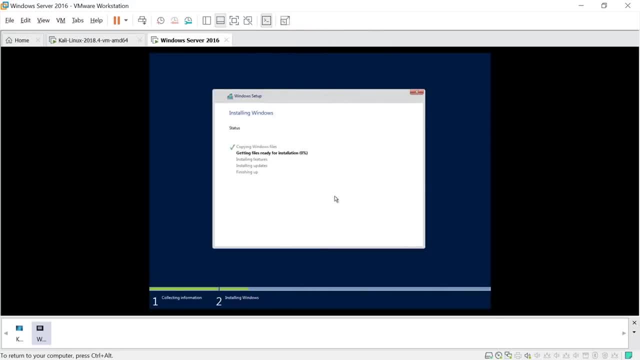 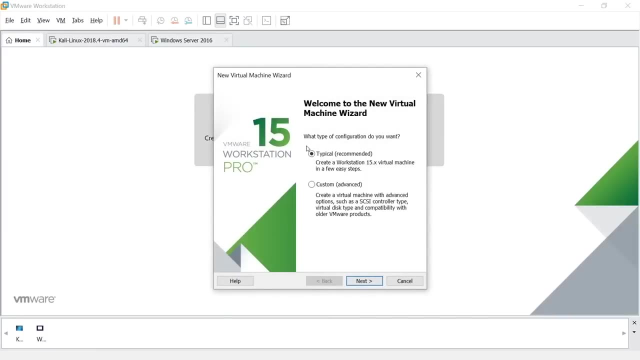 Okay, so let's let this install. This will take a few minutes, Not too long. While this is installing, we're gonna multitask just a little bit. We're going to create another virtual machine. Again, we're going to say: typical. 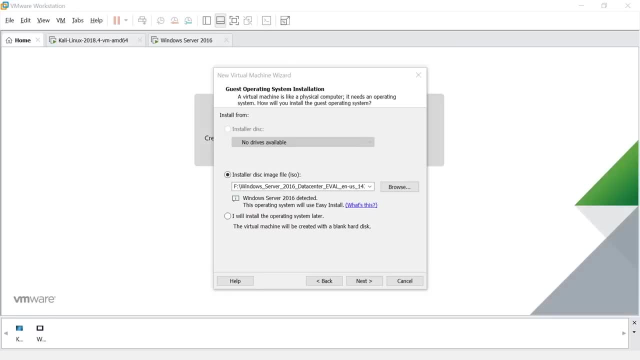 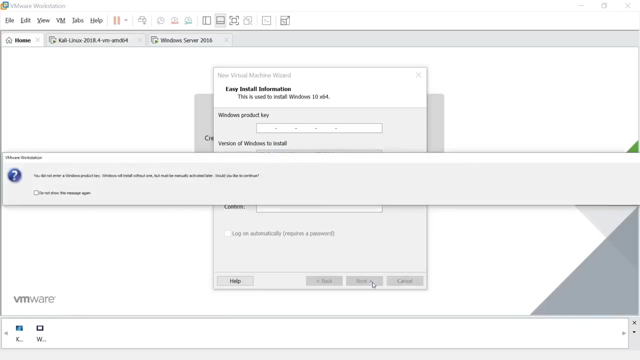 And I've got this copied for the other ISO. So select your Windows 10 ISO and it should come up: same thing: Windows 10 Enterprise. hit next, hit, enter again. I have a server for this or a folder for this. I should say: hit next on this guy. 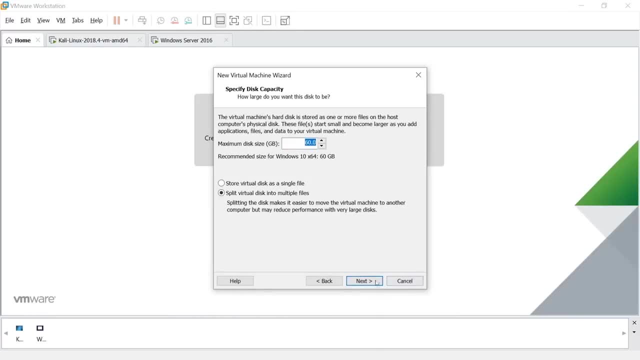 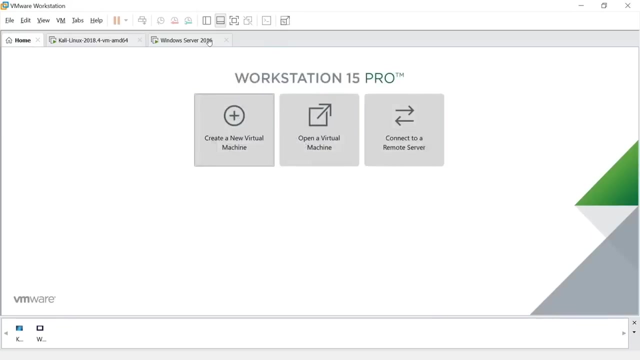 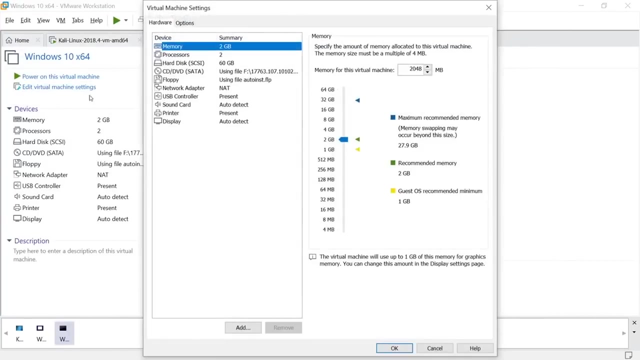 same thing: 60 gigabyte file. I'm gonna hit next again. we're not gonna power on the virtual machine after creation because same thing here. it tries to install that floppy disk and you can see things are starting to run a little bit slower. and that's okay, we've got time, so let's go ahead and remove this floppy. 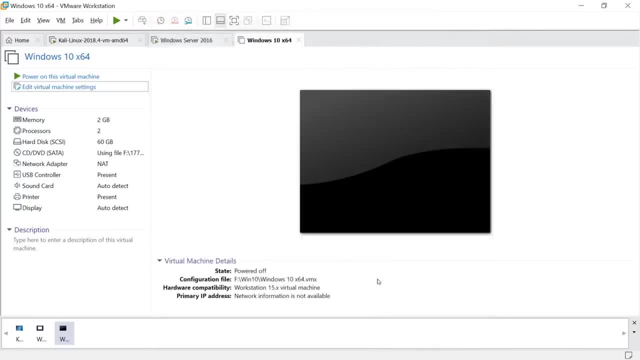 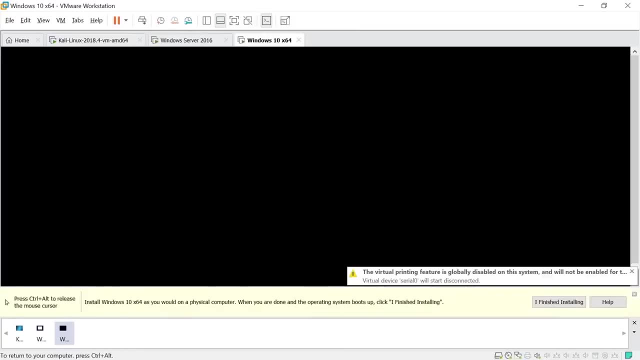 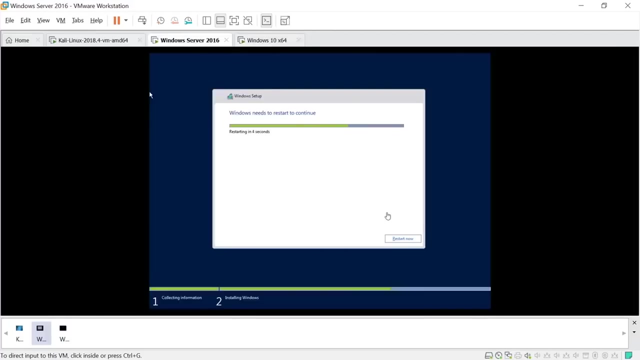 disk again hit. OK, and we're also gonna power this guy on. get our fingers ready, hit our key there to get it running clothes out of this. okay, you're window setup will automatically restart. we're gonna try to multitask to just speed this up a little. 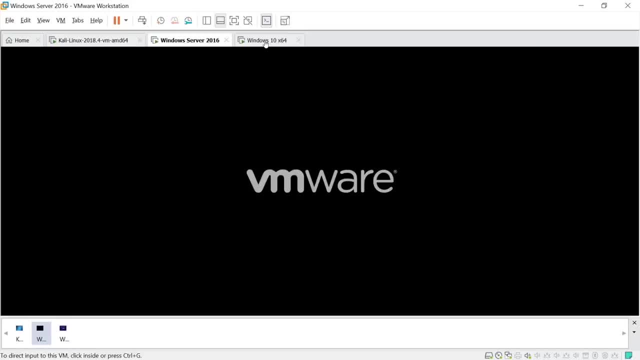 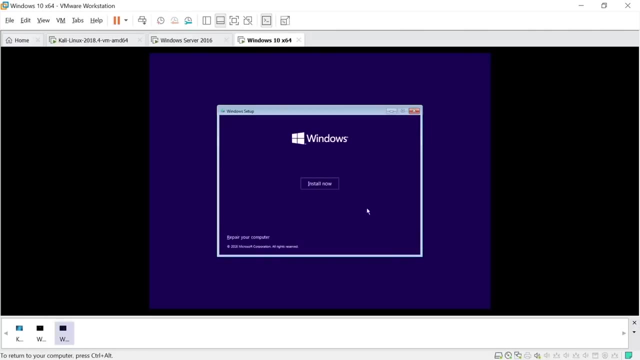 bit tonight. I've only got one lesson plan. so if we, if we finish early, we finish early, everybody gets go to bed sooner or stay up and party, whatever your prerogative is. so on the Windows 10 side, gonna go ahead and hit next install. now MTX was complaining to me earlier that this was going to be boring, and he 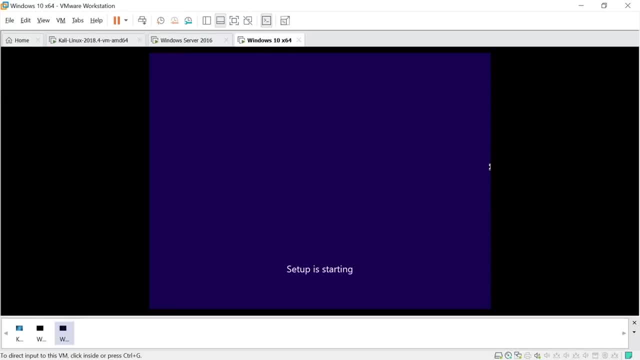 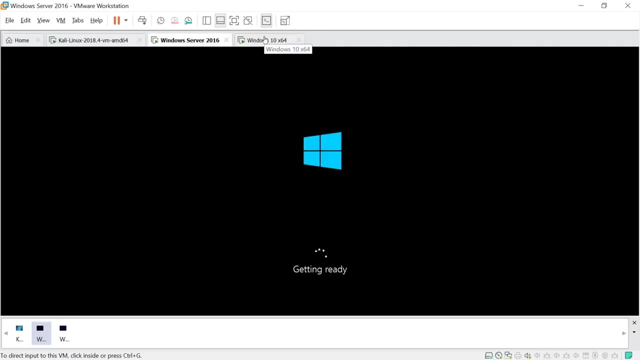 wasn't going to be here to enjoy this, but look, he showed up. the basics are important. you've been up since 430, Jeff. you're living that Air Force life, my friend. all right, if your window setups ready, accept the license terms. you've been up since 430, Jeff. you're living that Air Force life, my friend. 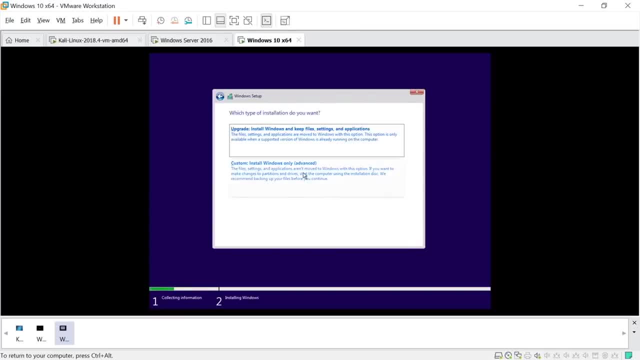 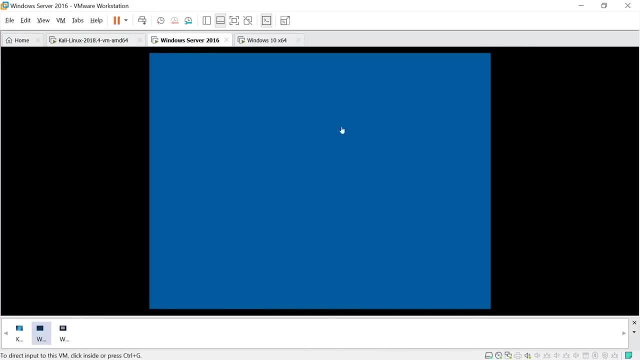 hit next custom install- again new on the bottom. it's the same concept. it's gonna create additional partitions for us because it's nice like that. it's gonna run through the same installation. server did all right, so customize settings. it's asking for a password on the web. I'm gonna be making my password the insecure password it has to have. 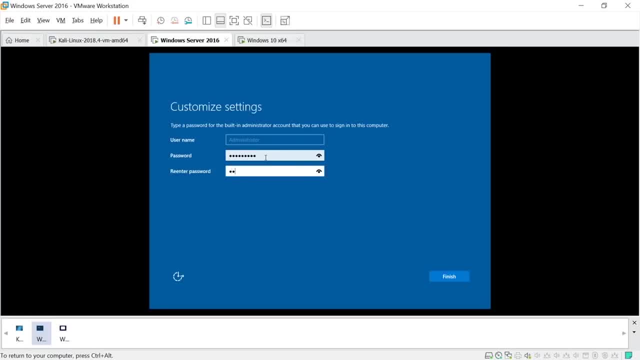 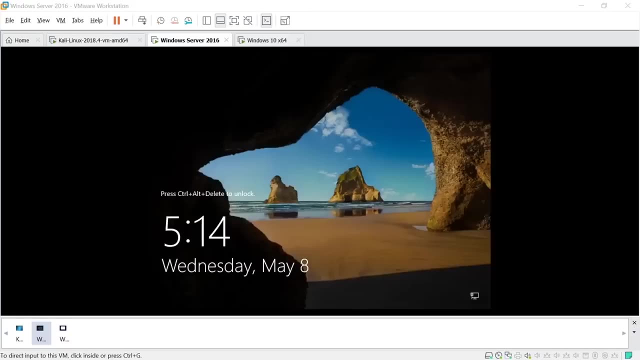 some uniqueness to it and I'll type this into the chat in a second, but it's capitalized p at dollar dollar lowercase w0, R, D, exclamation, hit enter. so if you want my password, if you want to use that, that's fine. if you want to. 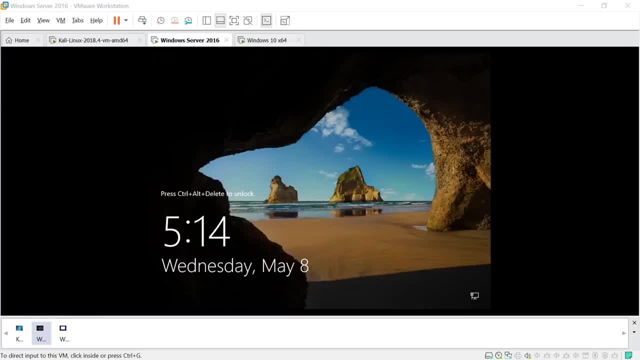 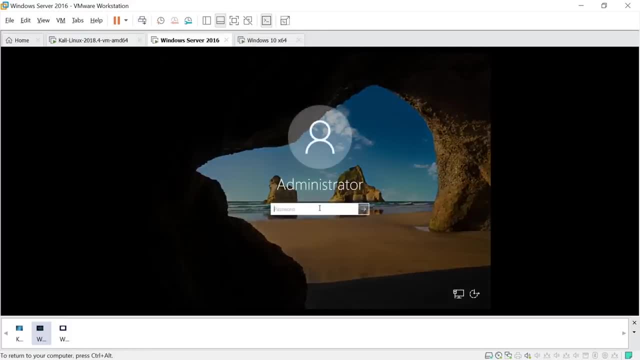 use your own password, do whatever, but for this instance I will make sure you do it. we're using password, as I just sent to chat. All right, send all control delete. We're going to log in as the administrator. Let's let that build a profile here. It shouldn't take that long. 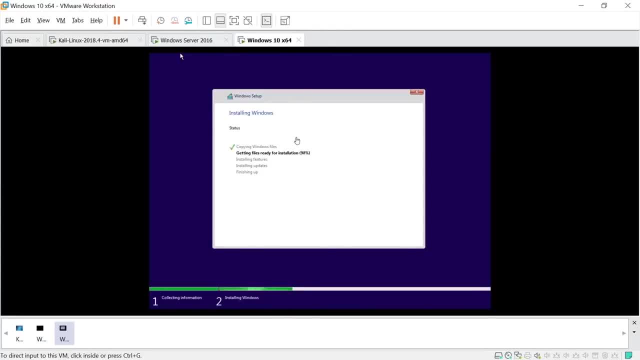 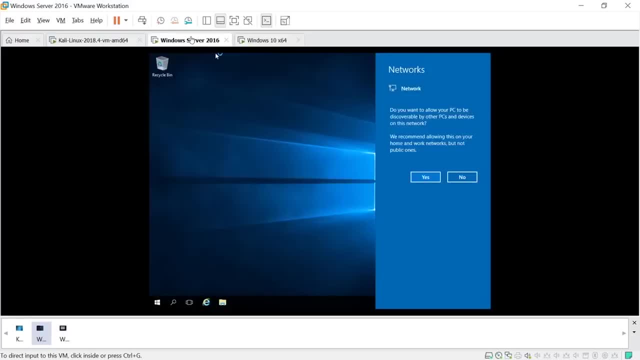 Windows 10 is going to be the one that's going to be fun, because it restarts and then Cortana starts talking, and we all know how we feel about Cortana. Do we want to be discoverable? Sure, we'll be discoverable. 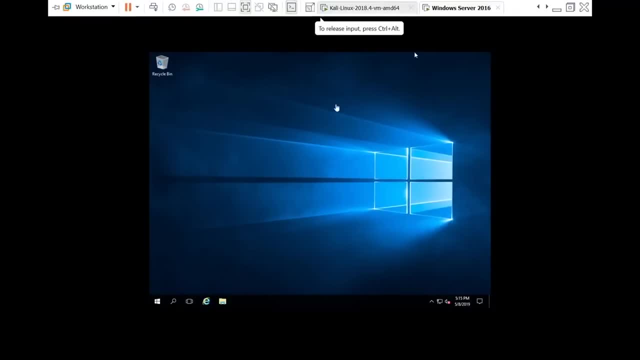 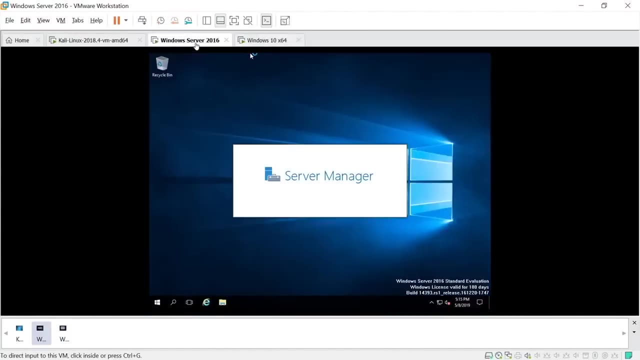 So we're going to have to reboot- most likely, Yeah- in order to actually get the full screen on this. that's fine. Okay, this is still installing, All right. so we're going to rename this server here in a second and do some settings, and then we should be good to go. 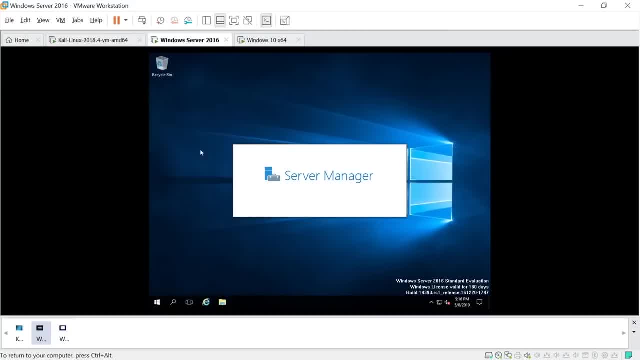 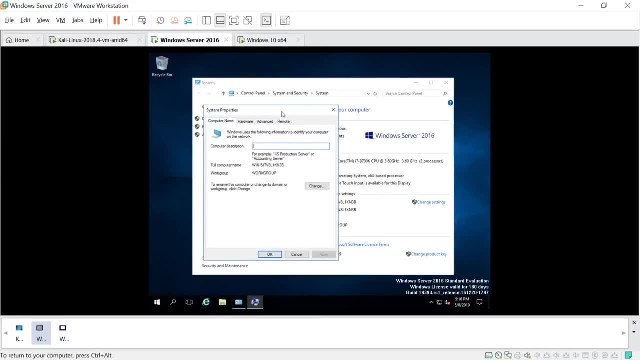 So I right-click, I'm going to go ahead and save this, I'm going to click on the little Windows icon and I go to system And we're going to change the name up here. I'm going to say change settings And then to rename this computer, change its domain, work group- click change. 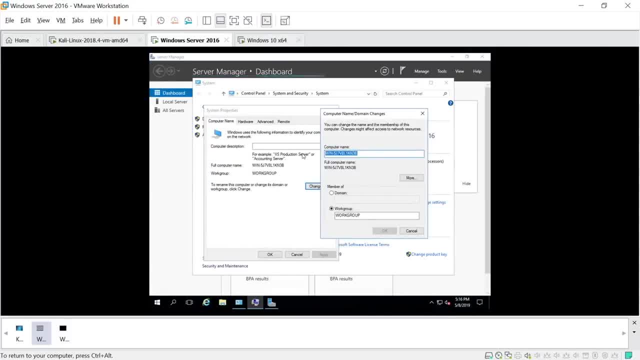 We're just renaming the computer right now, So I came up with a theme for this. The theme I'm going to be using is the Marvel universe, So we're going to be calling the domain controller Hydra, since there are a bunch of evil hacker people, et cetera. 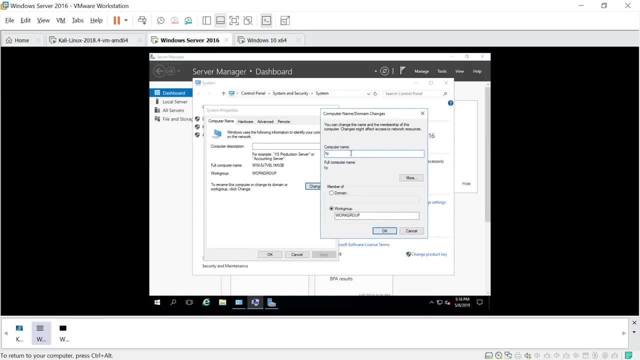 And we're going to try to hack into Hydra And we'll create some fun people along the way. but let's rename this Hydra. Let's use it as an excuse to reboot the machine and hopefully get to full screen on this sucker. You can see how slow things are going. That's okay. 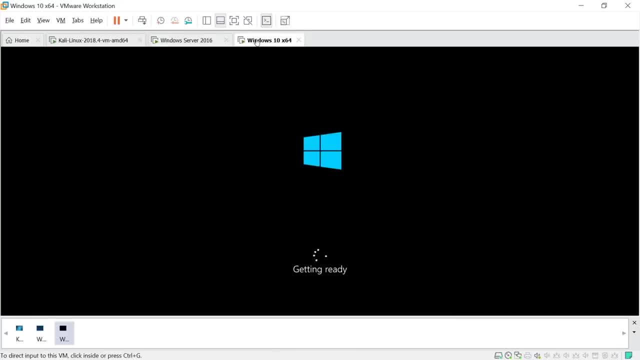 Restart now. Windows 10 is going to get stuck in getting ready for a while. Cortana will just pop in when she feels like it pretty much what she does anyway. All the accounts in your Sans course were named after Marvel characters. That's awesome. 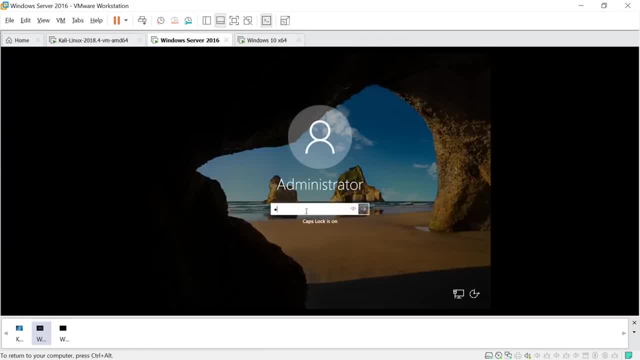 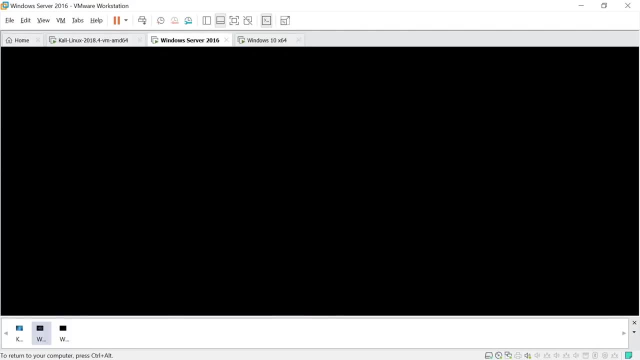 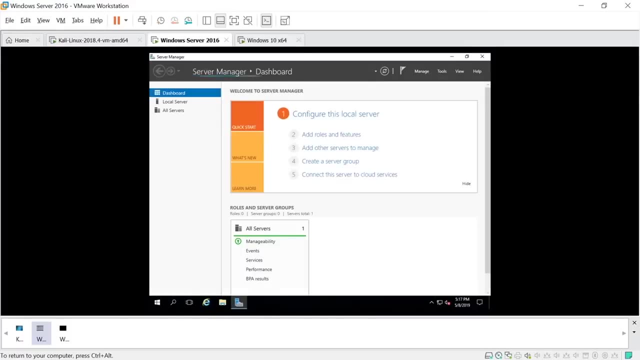 I'm not a DC guy. I do like Batman. I do like Batman, though If I'm going too fast, please, please, slow me down. We've got nothing but time tonight, MTX, you're lost, Bro. you're the one telling me that this was easy stuff. 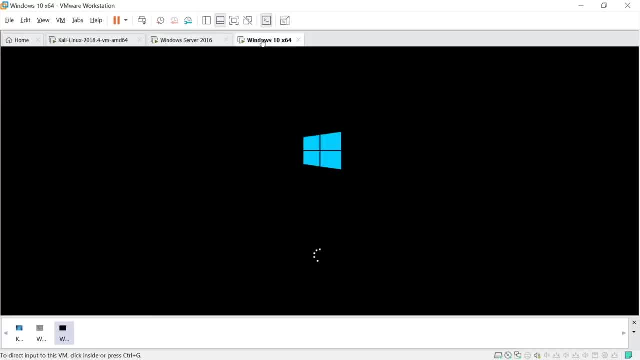 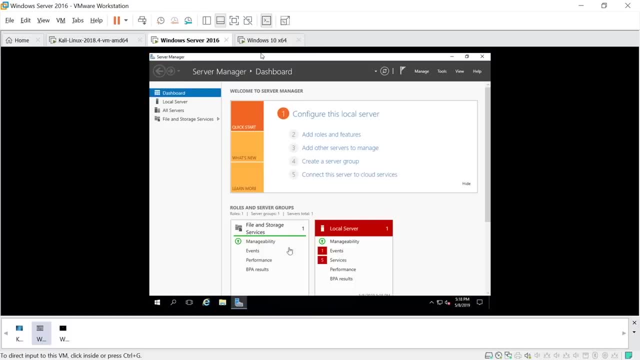 Why do we need this lesson? Because I'm the only one today. I renamed the- the domain controller to Hydra- As myame. I need to go to the game because I'm so busy. I had to take my own time and do my own thing, and I can't just sit and do this. 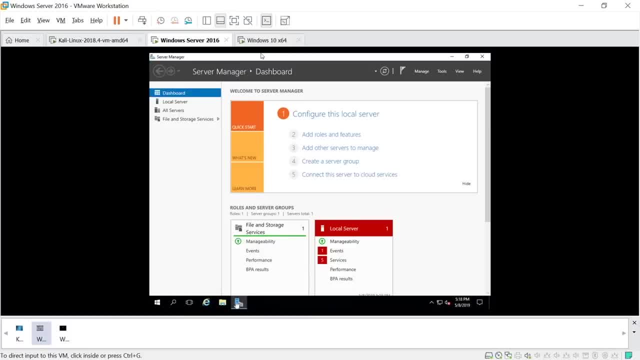 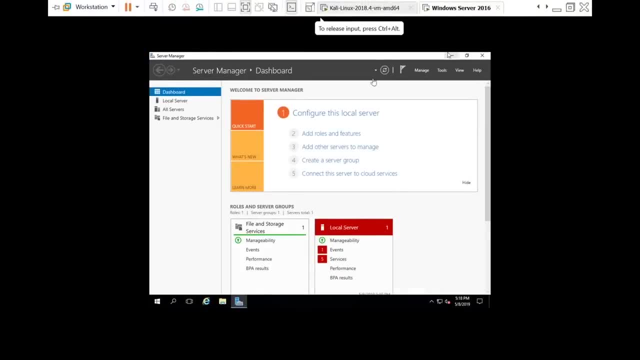 My name is Jambor. You can rename it whatever you like. I'll just do it when you're done here. I… I guess I'll have to do this one after the game. I won't be able to do it if I don't choose to do it after this, but I'm going to try again. 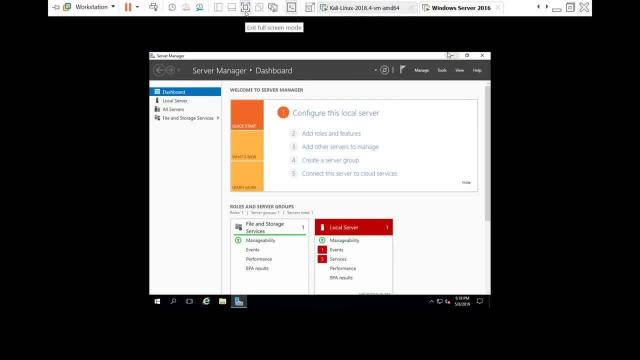 You can rename it whatever you like. If it's not in my favor, then I won't. Let's just give it a try. I'm not that good at this game. My name is Shane. You can rename this controller to Hydra. 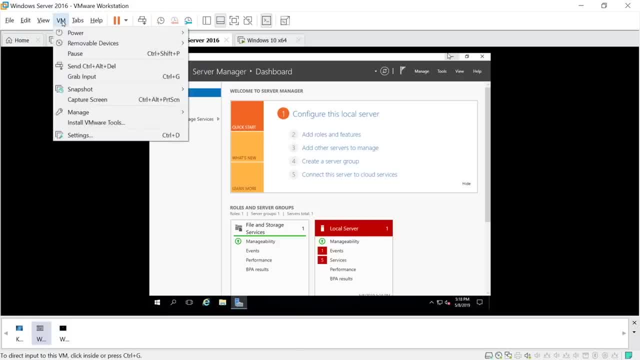 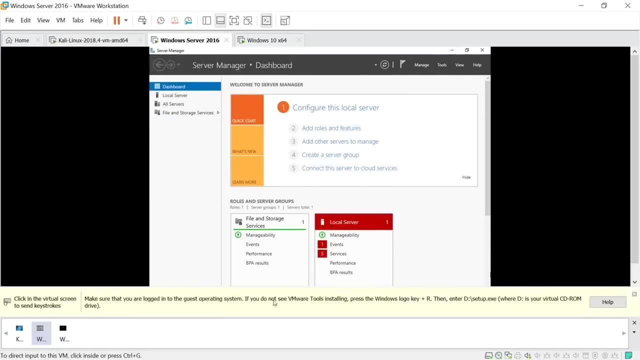 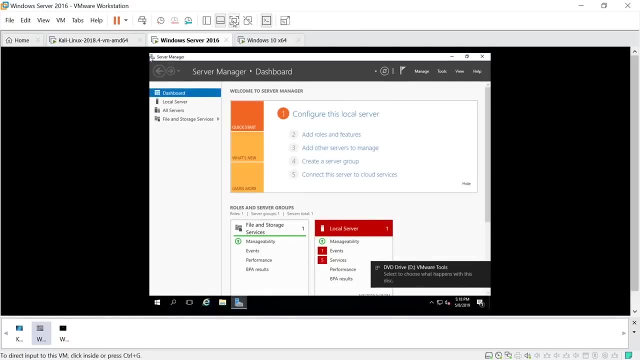 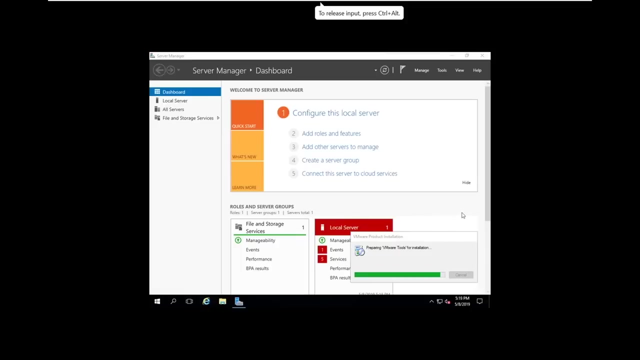 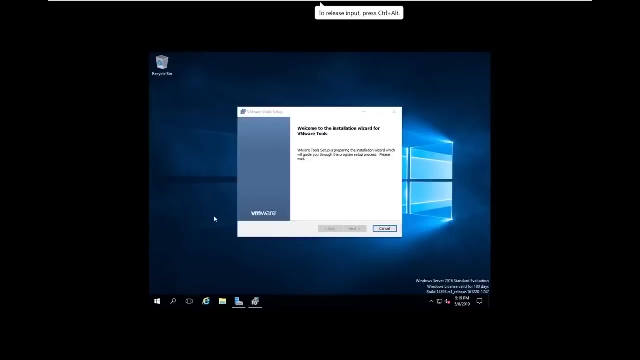 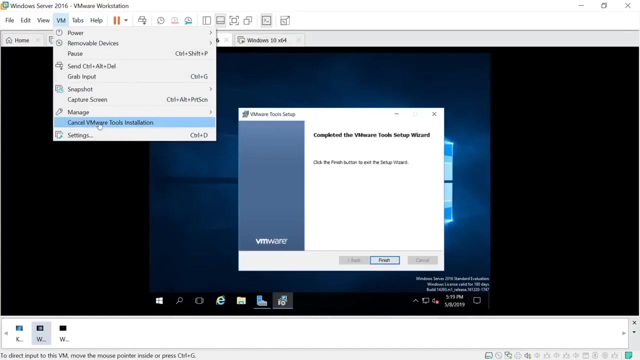 we may have to install VMware tools. maybe don't know if it's worth it. it's not worth it for tonight. let's see. this requires the full reboot. we'll see. we'll do a complete install. install. you guys didn't see that. there is a VM up here and it says: install VMware tools. just do that. 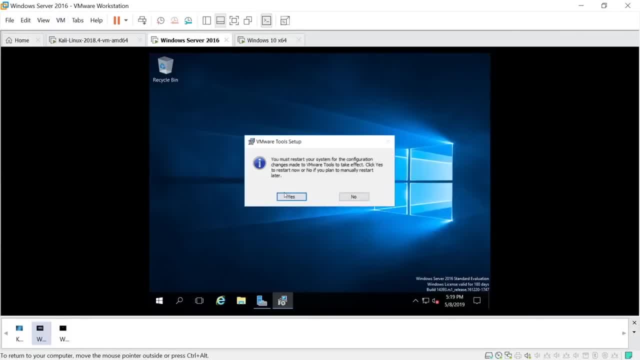 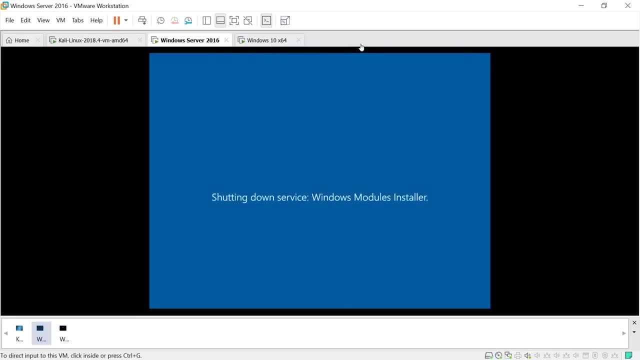 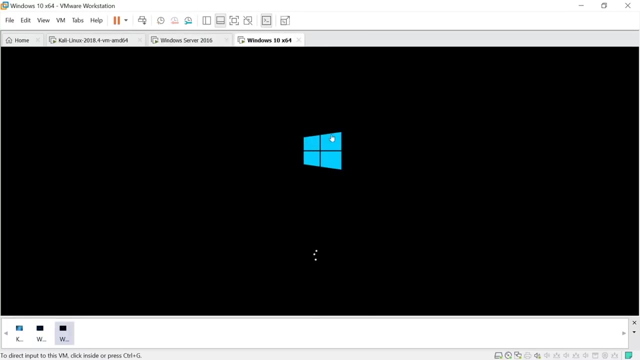 okay, reboot the machine. MTX. no more questions. we'll get out of work group. when we're out of work group, your Windows 10 should still be spinning. you can install server 2016 faster than you can Windows 10. let that be a life lesson. 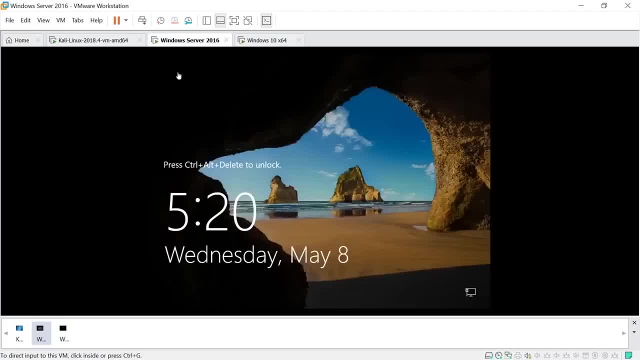 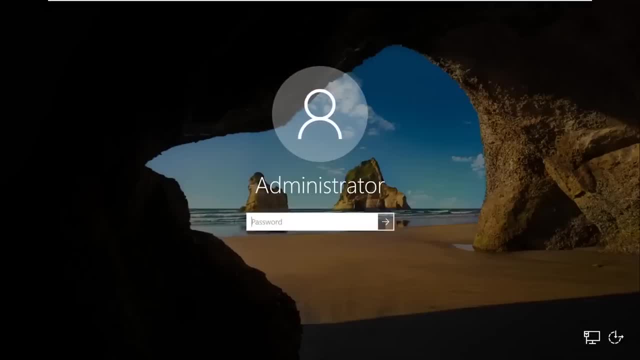 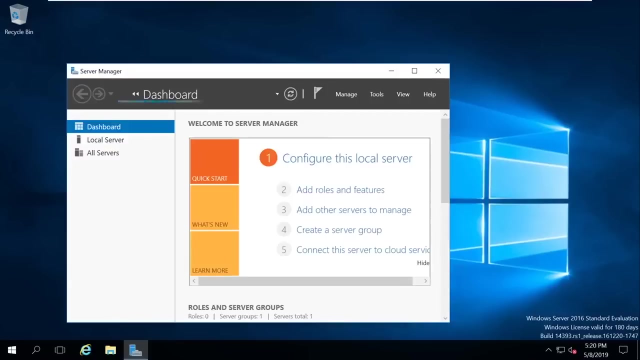 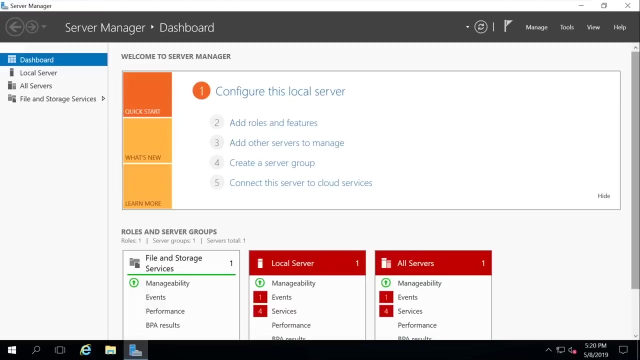 for you. let's see if this worked. ayo, alright. so while we still wait for Windows 10, we are going to start working on our active directory. somebody said their server is just finishing up its install. i will go as slow as possible and drag this out just a tad, if i can. hi there, i'm, oh, there's cortana here to help. we can stall. 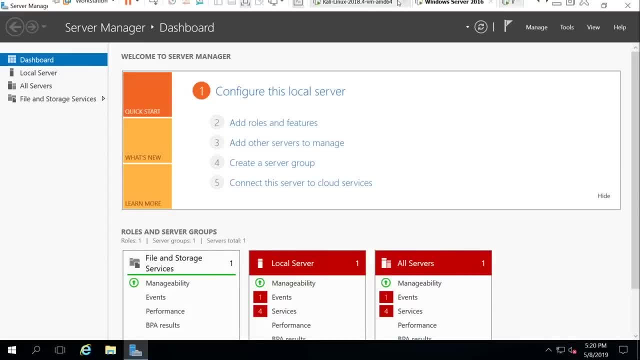 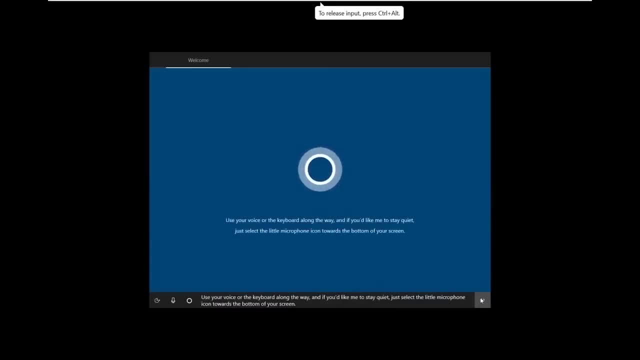 just a little bit. sign in here, a touch of wi-fi there and we'll have your pc ready for all you plan to do. use your voice or the keyboard along the way. let's mute her, like me to stay quiet. just select the little micro. there we go. 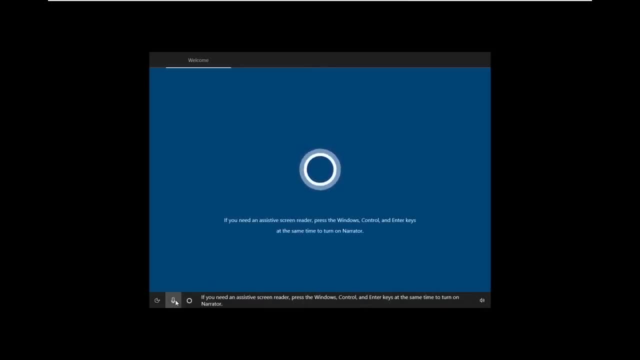 tick tock, tick tock. all right, start with your region. i'm in the united states. we're going to start with the united states here. this is keyboard layout. right, yes, skip the second keyboard layout. i'm unsure how long this part takes. we still have to log in, go through the hello screen, all that fun jazz. 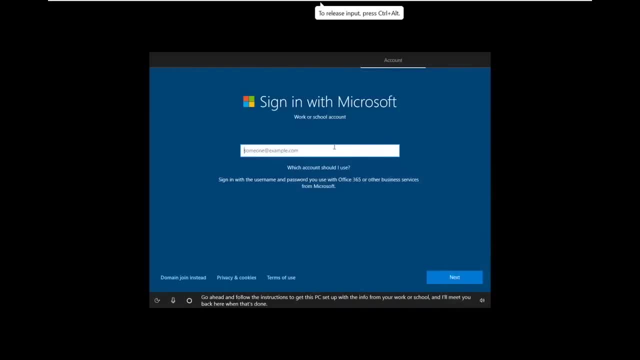 oops, didn't mean to bring that up, all right. so we're going to go down here and say: domain join. instead, that's just going to let us create a, an account. so i'm just going to name this one frank for the account. local account. create a super memorable password. uh, all right. 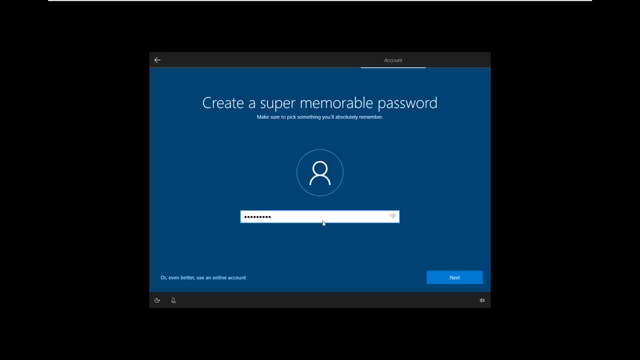 what should we name it? password one, let's see if it lets us do that. it does so. password one with the capital p, nothing insanely complicated. that'll come into play later. we have security questions. that's fun. what's your first pet's name, bob? uh, what's your pet's name here? 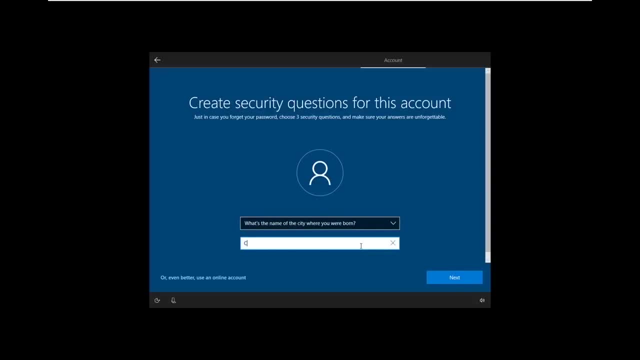 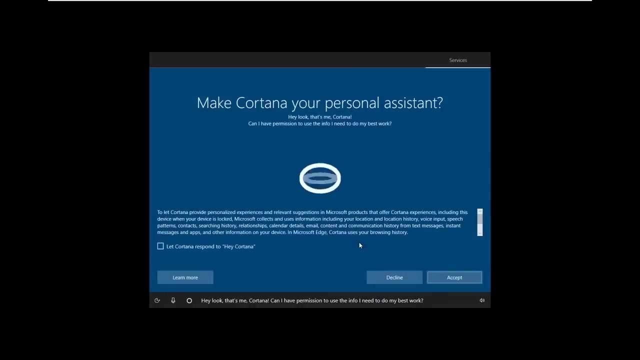 uh. what's your pet's name here? ummyfrench's. uh. uh. what's your pet's name here? uh, what's your first pet's name here? where do we grow up? we'll say we grew up in Chicago. and what's your childhood nickname? we'll say our nickname was bobbert. if I could spell it, do we want? 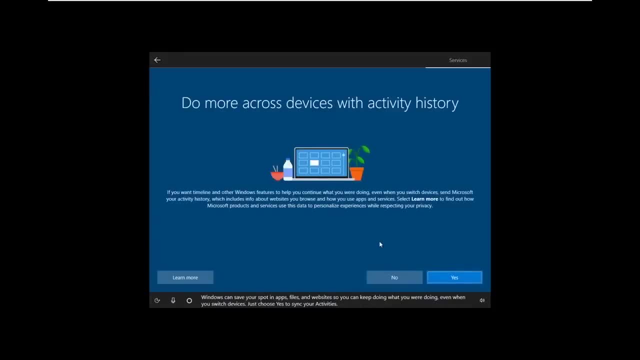 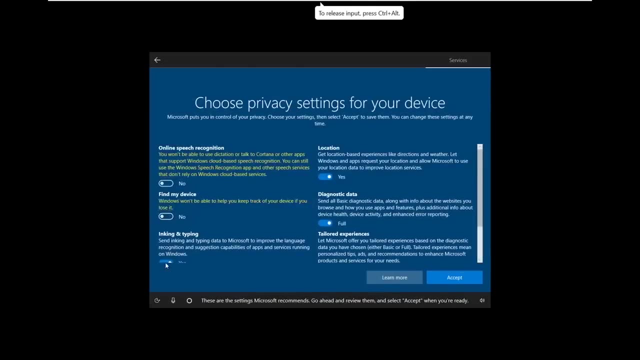 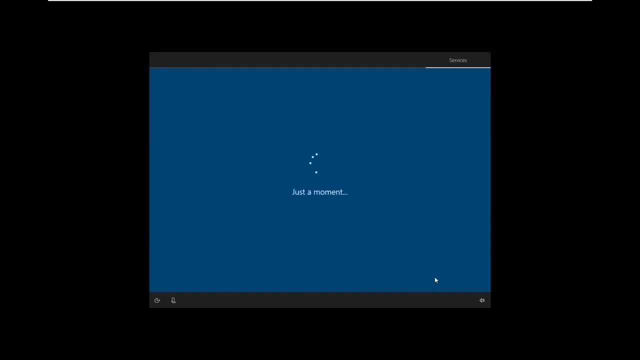 Cortana- hell, no, we don't want Cortana. decline no activity history. look at all the stuff it wants to just spy on us with guys. you don't want any of this. hit accept. turn that all off. and hit accept: okay, we'll let Cortana do her thing and it's gonna go through this whole screen. 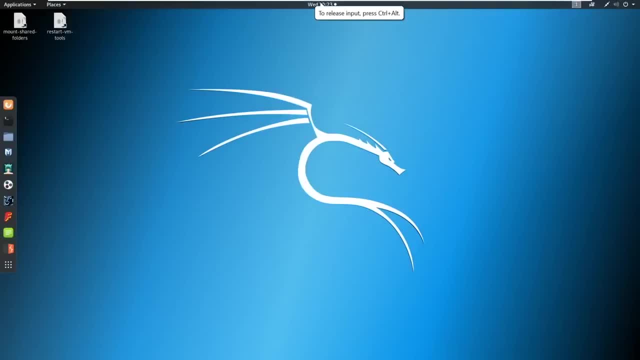 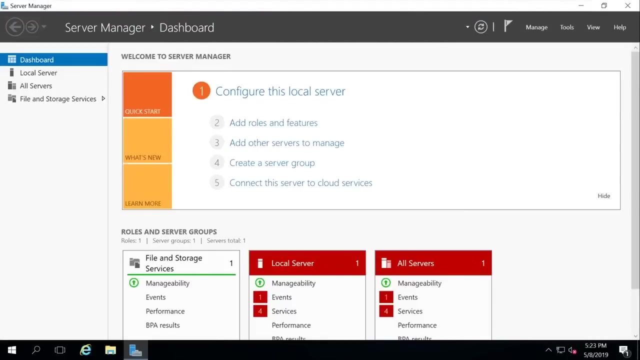 so, while it's doing that, let's- uh, let's- install- sorry, I went to my Cali- go to server 2016- let's start working on setting up our domain. so first thing we're gonna do is we're going to say we're gonna be in the server manager. that should have popped up on start. 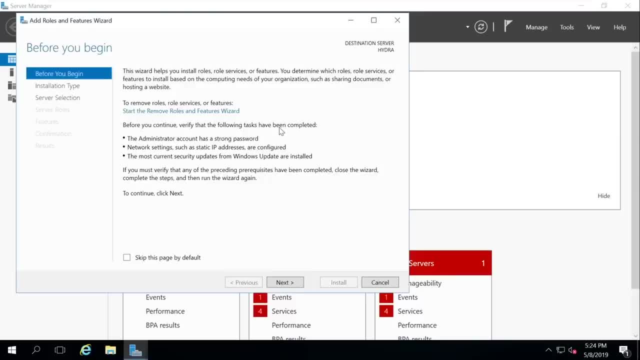 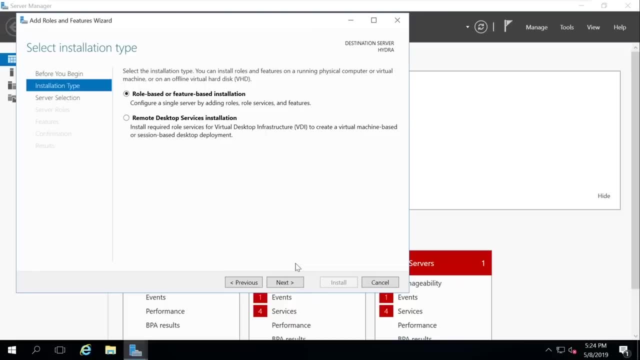 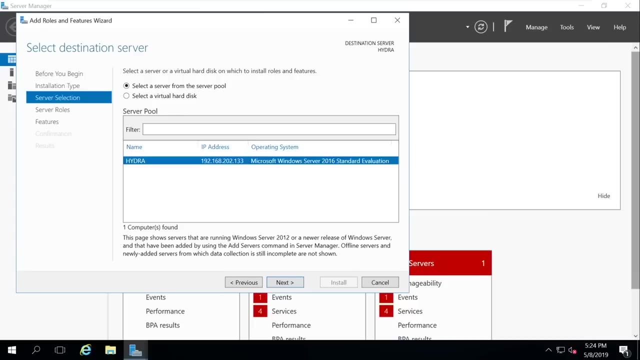 you're gonna say add roles and features, it's gonna give you this little wizard: just hit next on this page we're gonna be doing a role based- uh, or feature-based- installation. hit next and it's gonna ask you to select a server from the pool. we're going to be selecting hydra. all right now, what kind of. 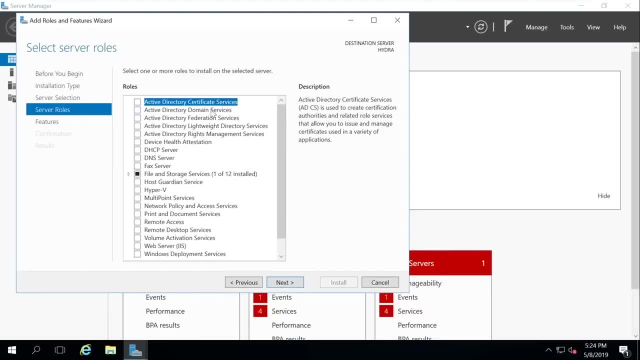 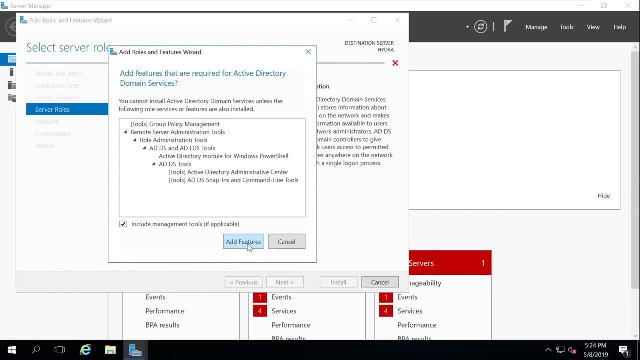 server roles do we want? well, we're going to be installing active directory domain services, so we're going to check that box and say add features and that should be it. so make sure again you aren't lol. nord uneachl exercises: read red email اخ. 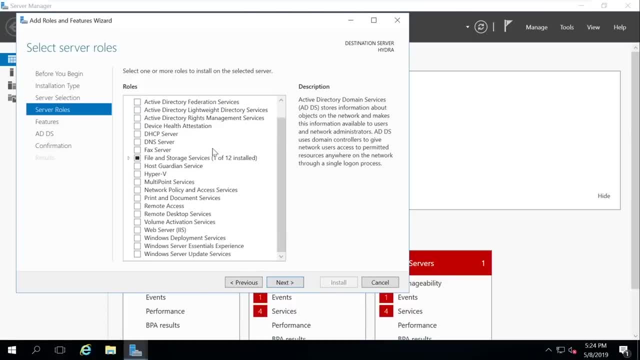 title: admin chrome pdf cloud, ezoi. check this box and hit add features. but this is where, if you wanted to add, like a dns server, dhcp, you want to add iis, for example remote desktop, you can come in here and add these features. okay, we hit. next. it's going to add group policy management. 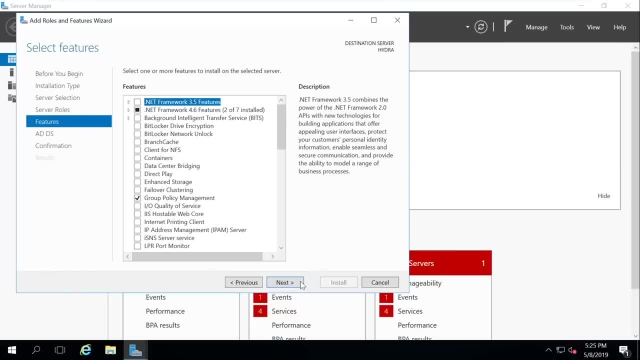 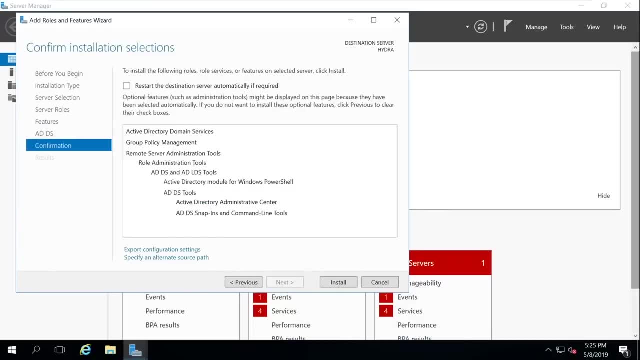 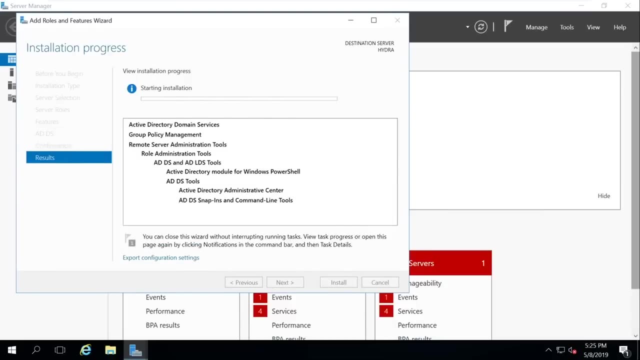 somenet framework. it looks like we can just hit next on that, next on the domain services, and then we are going to just hit install. so this is going to take a second to install and then we're going to have to promote the server here in a second. 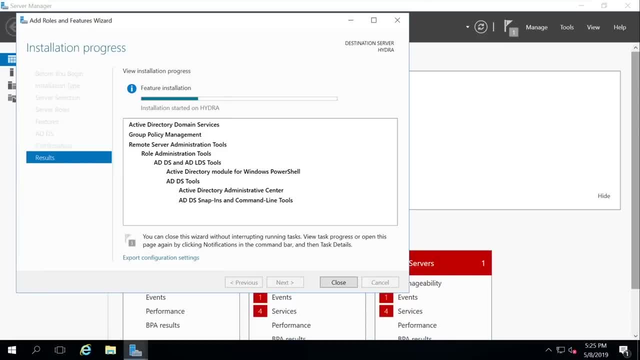 should name the controller red skull and use hydra for domain. yeah, that'd be a good idea. we're just going to use marvel for the domain. all right, looks like we are done here. we're installed. i'm just going to hit close. you see, we've got a little notice up here. 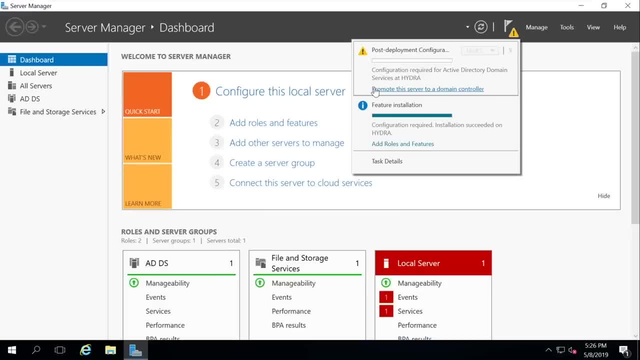 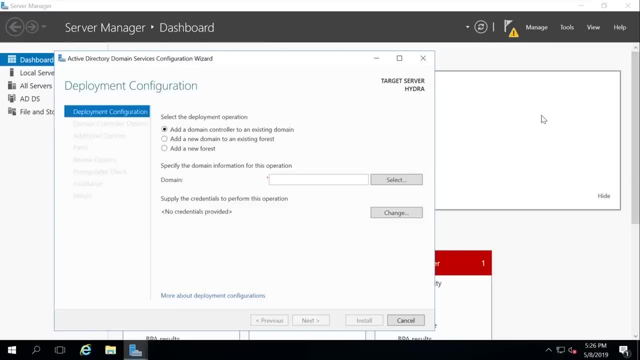 and post deployment configuration. promote this server to a domain controller. we're going to click that, all right. and then we have some options: add a domain controller to an existing domain. we don't have one. we don't have an existing forest, so what we're going to do is create a new forest. 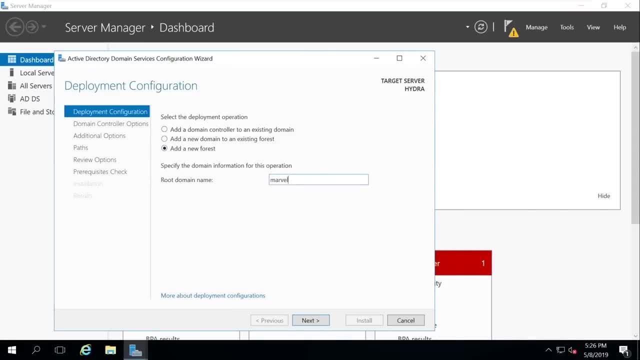 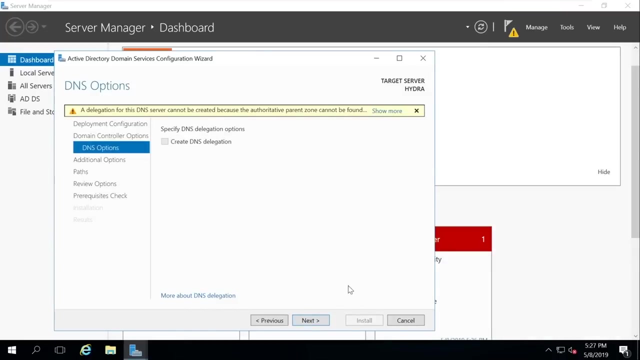 and we're going to call this marvel dot local. hit next might take a second. okay, windows server 2016: perfect, we're going to have a directory services restore mode. we're just going to use password again because we're terrible admins. okay, hit next. leave dns delegation blank. hit next. 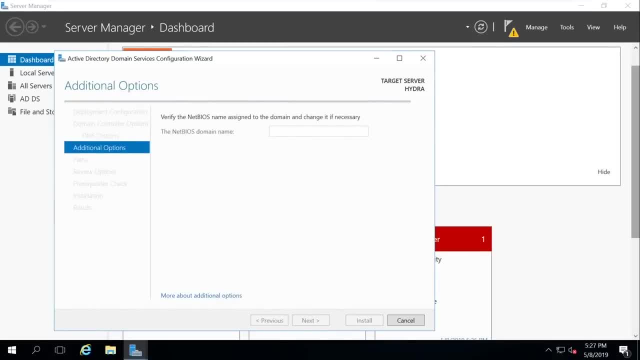 it's going to generate the net bios name. it should be marvel. takes forever too fast. i will slow down. where are you stuck, morse? help me, help you, sir. thank you for the cheer- anonymous cheer. it's here, see if somebody can help me. ok, i'm gonna call another server. 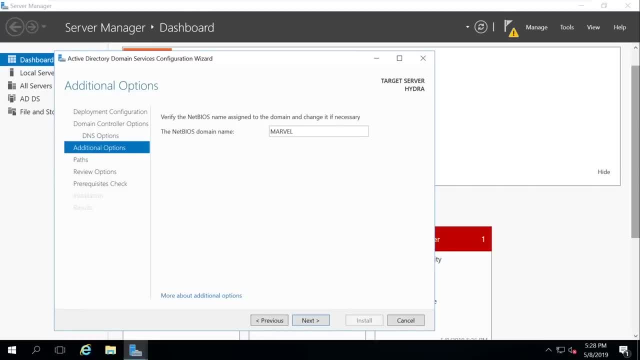 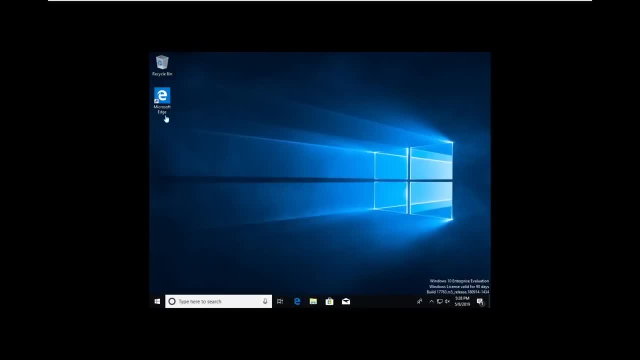 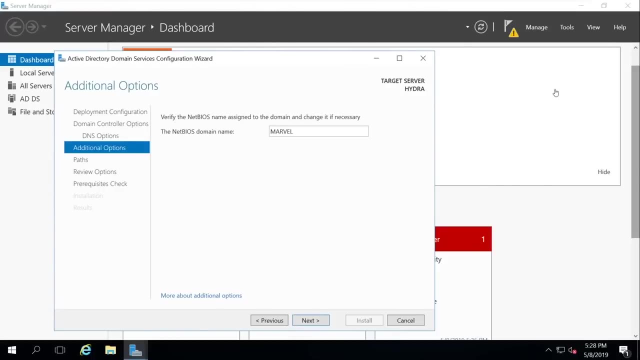 install the server earlier for YouTube video. Windows is just now finishing. ummm, that's fine. we're we're not touching Windows 10 yet, so Windows 10 should be logged in like this. we're just touching windows 2016, the server 2016. 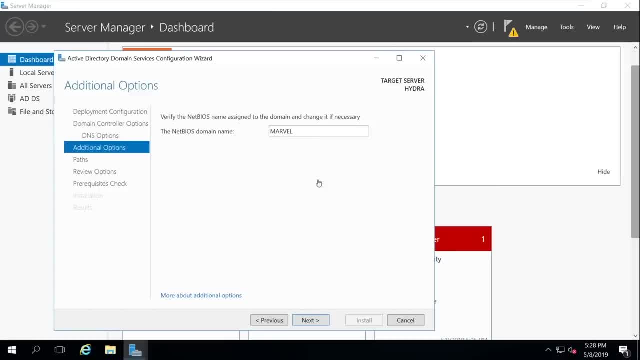 in the server 2016, All right. so with Marvel here, once it populates in the NetBios domain name, we're going to hit next. It's going to give us the paths for the sysvol and stuff here in a second, the NTDDS maybe. 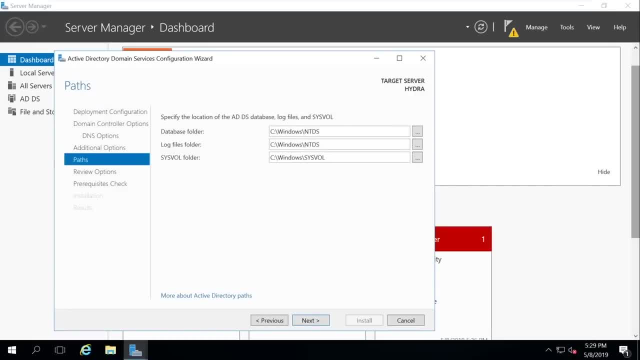 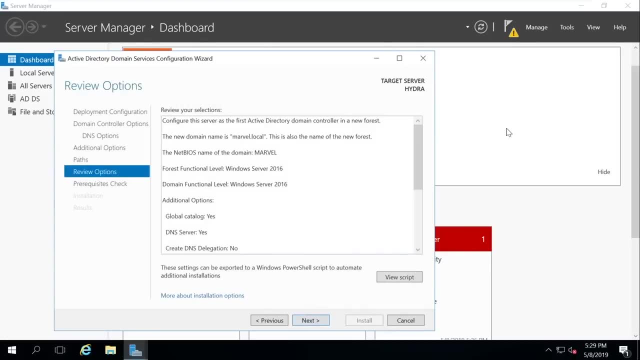 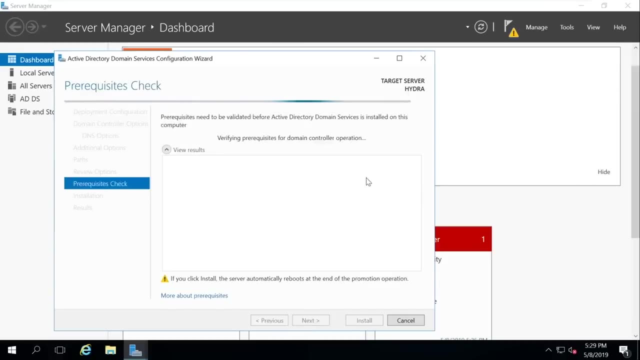 Okay, So leave these on default. Let's hit next. We're going to go ahead and just accept all of these options. We're just reviewing the options This is going to populate. We're just going to hit install Someday. 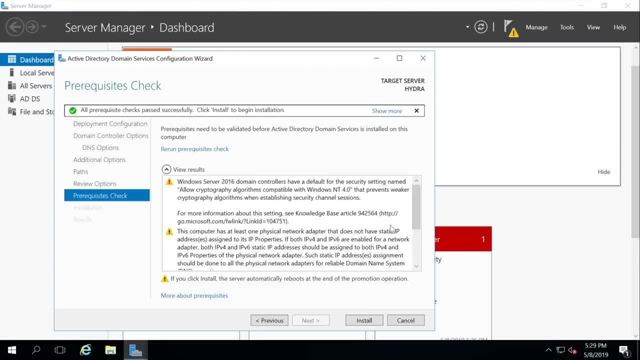 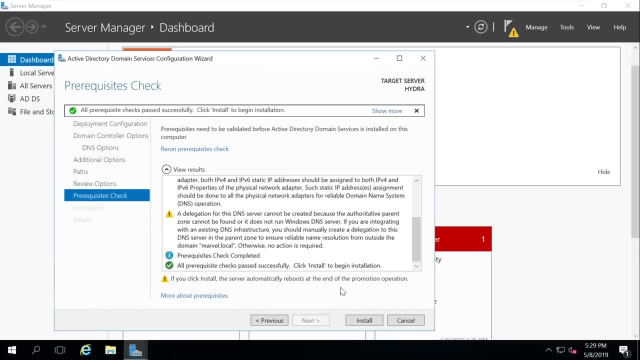 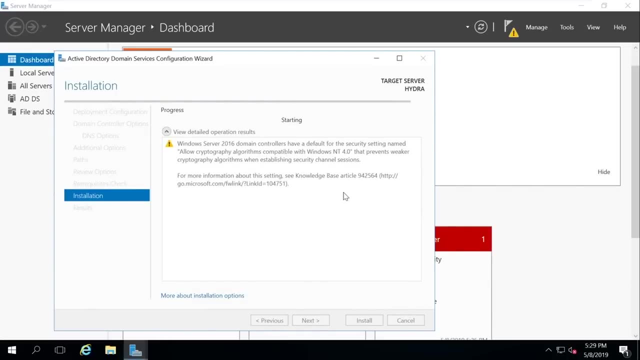 Okay, All right. So basically all it does is a prerequisite check to make sure that you can make this a domain. We pass that check, We hit install. It does the installation. This will take a little bit of time and then we can join our domain controller with our. 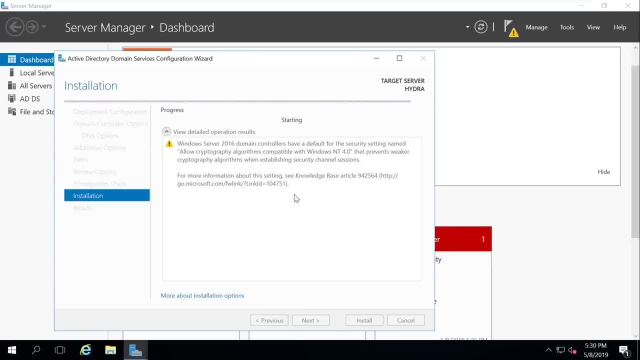 Windows 10 machine. All right, All right. So tonight is only going to be one lesson in terms of exploitation: We're not going to exploit too much, We're going to carry on into more exploitation next week. Is this only possible with Windows 10 Enterprise? 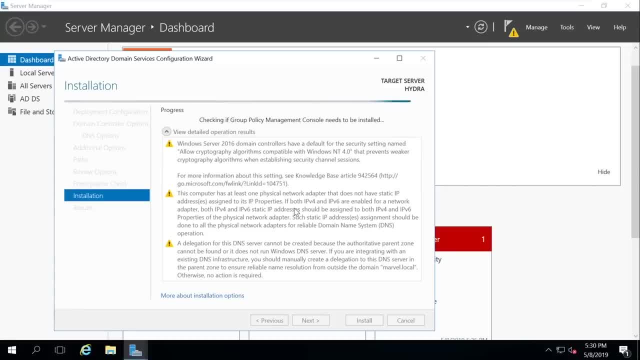 No, this is possible with Windows 10 Pro as well. I just don't think Windows 10 Home. you can join us and then you can use Windows 10 Enterprise as well. The only thing I think that's going to be very nice about that is the fact that we're 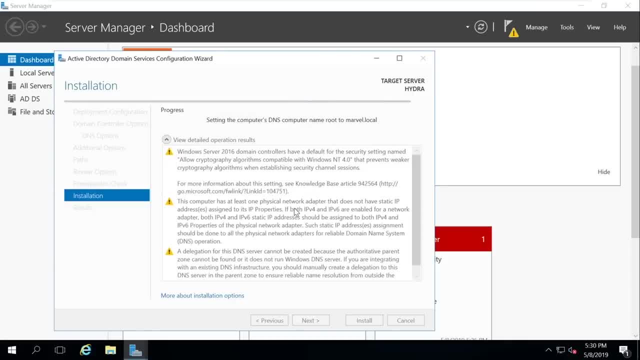 still working with Windows 10 Enterprise, We're going to be in a better position than we were doing in the past. I think that's why I'm happy that the Microsoft Office and Jingle Will do this, but it's great that the Microsoft Office has already made this possible. 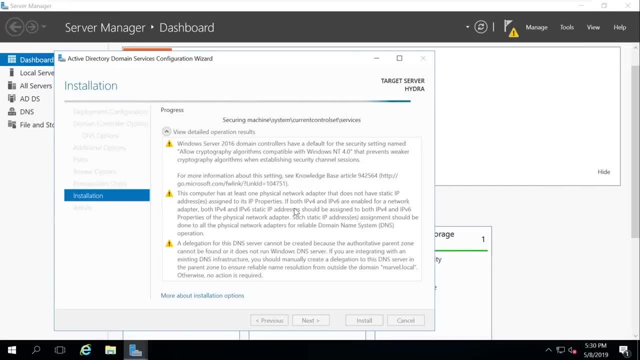 There's only one thing that's going to be a good thing about doing this. The great thing about this is that we're not going to be a big part of the company and Enterprise. No, this is possible with Windows 10 Pro as well. I just don't think Windows 10. 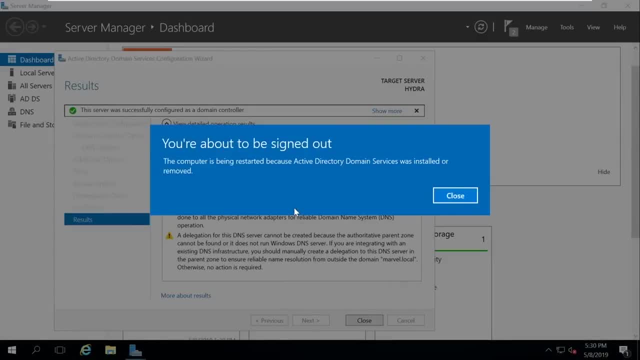 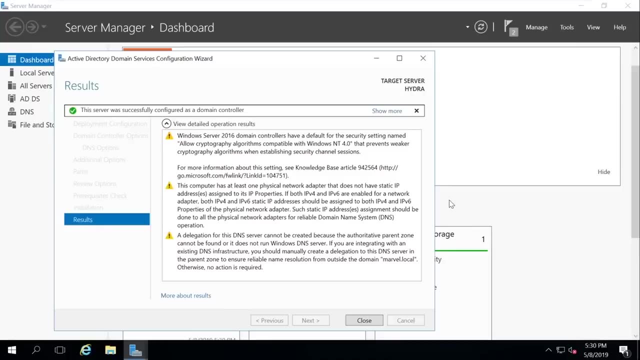 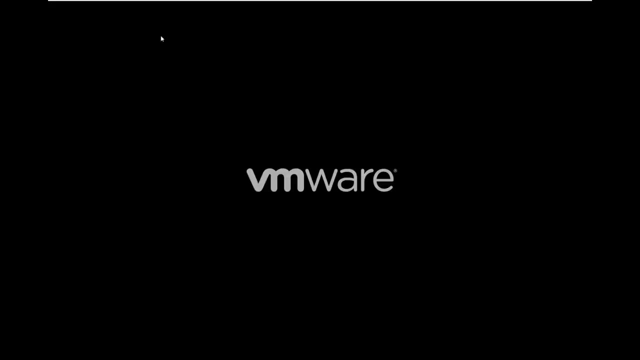 Home you can join a domain. So whichever ones you can join a domain with, I believe Pro and above- Okay, you're going to get signed out. It's going to restart the machine. Congrats, Solo, you got your cert in a week. 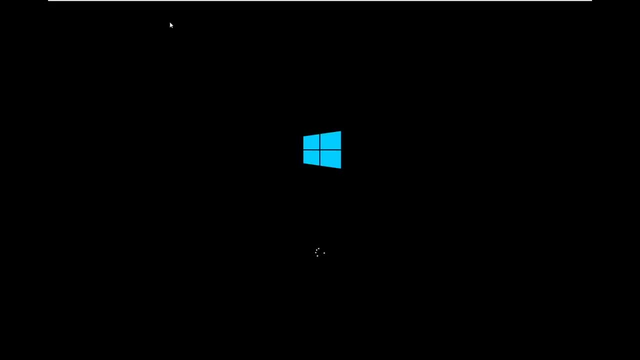 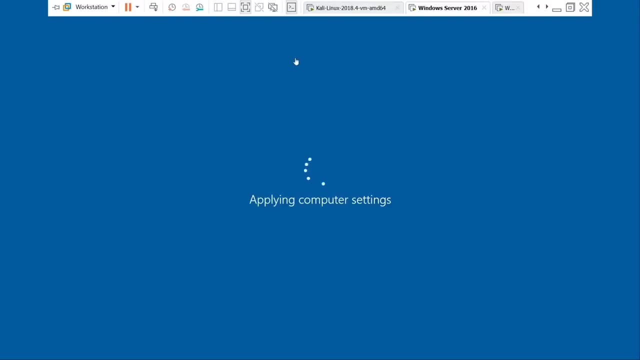 That's pretty impressive. I enjoy the EWPT. That's a good one. I have to take the WPTX exam in one week. I'm just thinking I'm going to delay it because I don't have time. Somebody said education can join a domain. That sounds believable. I'll take it as I. 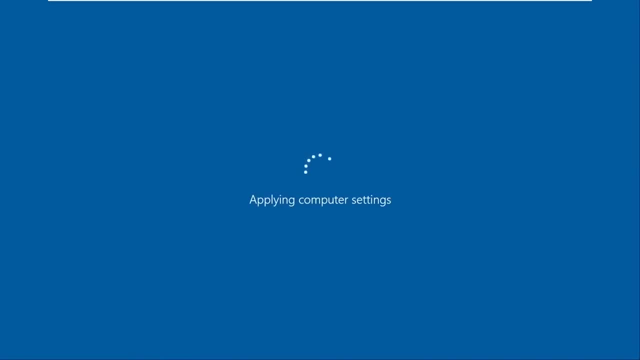 believe it. So we'll let this apply the settings And you guys can ask me questions while we're waiting. We don't have to have dead air. If you've got AMAs or I'll start picking AMAs, All right, I've got AMAs from the CyberSec Lounge that I can pull from, So if you guys 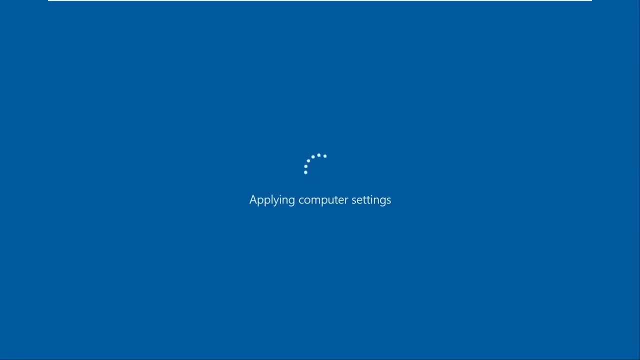 didn't hear the news. the CyberSec Lounge, Davey, has stepped up. I'm going to take a step away to focus on family. So he handed over server ownership to me a couple days ago. I'm running that server as a mentor capacity. Really, it's run by the mods over there Prior. 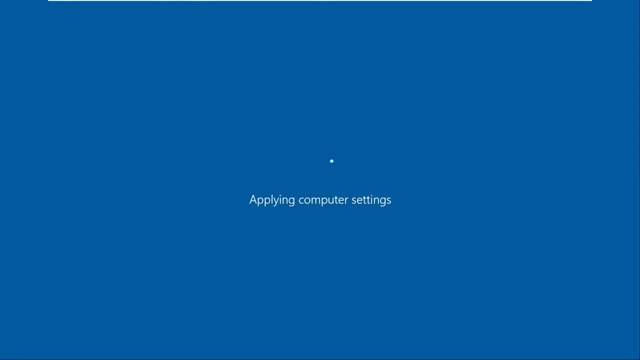 to his stepping down. we were going to be doing an AMA tonight And that did not happen because it would be weird to AMA me as coming in as an owner. So instead I'm going to take some of the questions and turn them into a video. 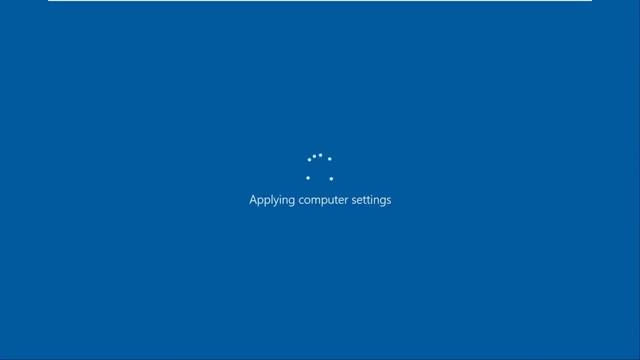 But I'm also going to pick some of these questions tonight, If we've got a little downtime while we wait and just answer some of those. Somebody just asked: why are we doing server 2016 instead of 2019?? There's no real reason. 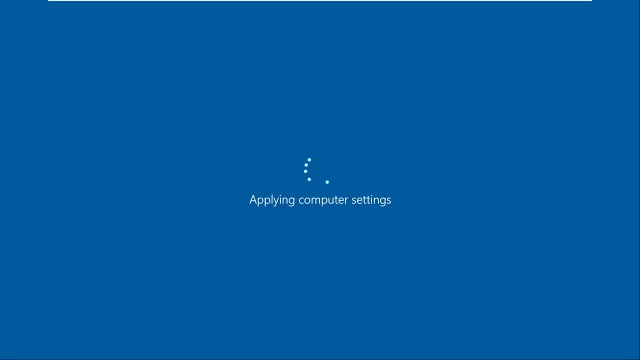 Server. 2016 is just more common right now, So we absolutely could do the same things on 2019.. I don't know what the little difference is. differences or nuances are between 2019.. I haven't got to play with it yet. So 2016 is more common. 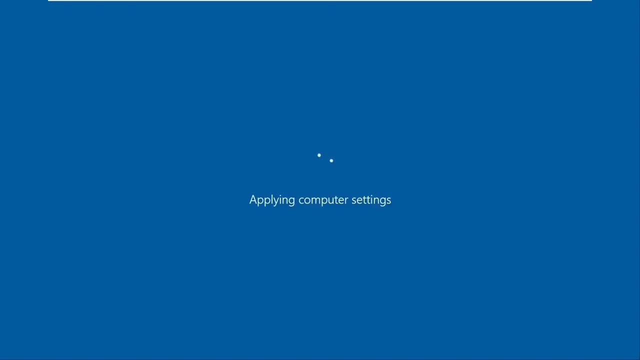 It's even really more common to see like 2012 still in a lot of environments. So it's better to use an outdated server when we're teaching this stuff, At least for the next three or four years. you're going to be seeing way more of 2016 than you are 2019.. That's just how it works. 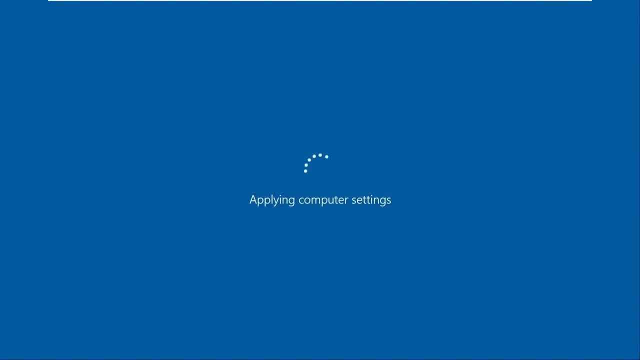 So when we spun up server 2016 and made a domain controller, didn't install Active Directory services by default. That is correct? Well, we didn't make it a domain controller. We made a domain controller when we turned on Active Directory services. So up until that point. 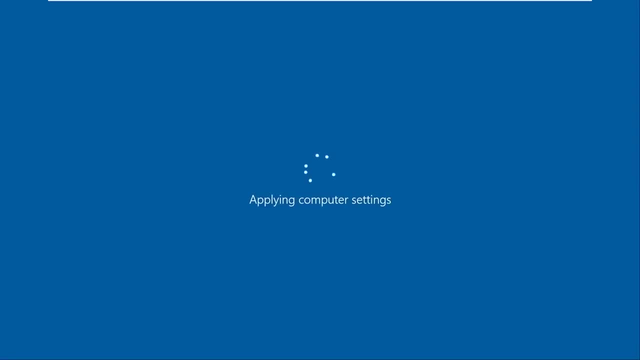 it wasn't a domain controller. We promoted it to one. Windows Server 2016 is bare bones. by default, Yeah, you have to configure it how you want to configure it. Terminal asked: am I going to DEF CON this year? I am not going to DEF CON with. 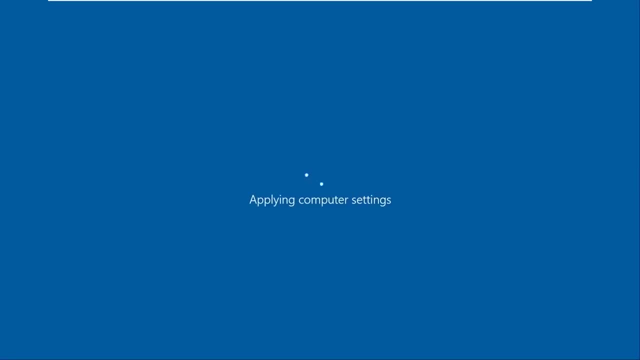 one caveat I apply to speak at B-Sides Las Vegas. If I get into B-Sides Las Vegas I will stay through the weekend And hang out, do LobbyCon at DEF CON and just chill, because I know a lot of people I know are. 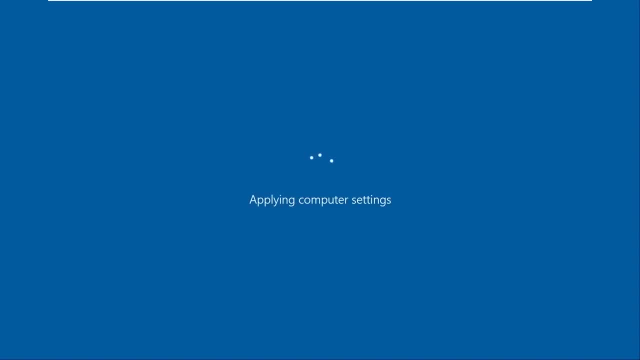 going to be there. So I'd like to definitely meet up with some friends and just have a good time. But so if I get into B-Sides Las Vegas as a speaker, then I will absolutely come out. If not, then it is what it is. 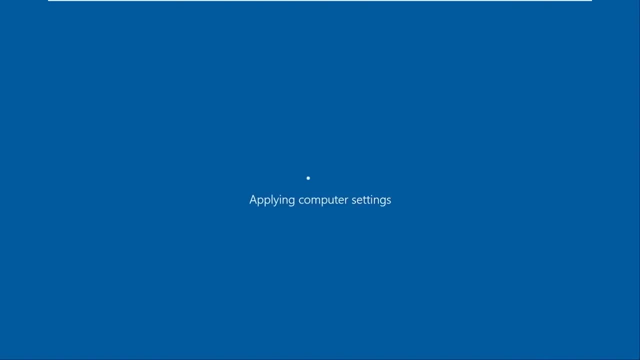 All right. So somebody asked Discount. Bin Laden asked: where do you get your news from? I mainly get my news from Twitter or any of the communities that I'm in, So really like being a part of quite a few Discord channels or being a part of BetSec. 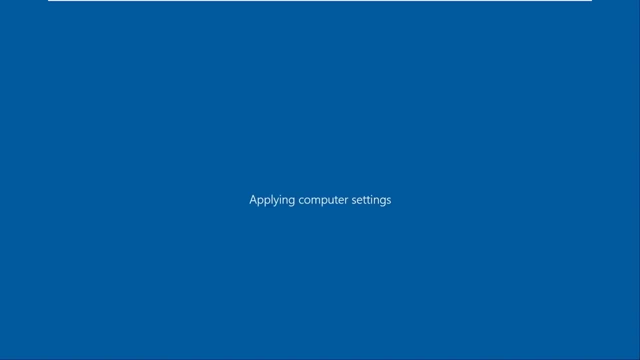 just joining those kind of channels that have categories for news. But Twitter is a really big one. Even news outlets are really big for cyber news. Ars Technica is not a bad place to get your news at as well, So it just depends, But mainly it's Twitter and communities. 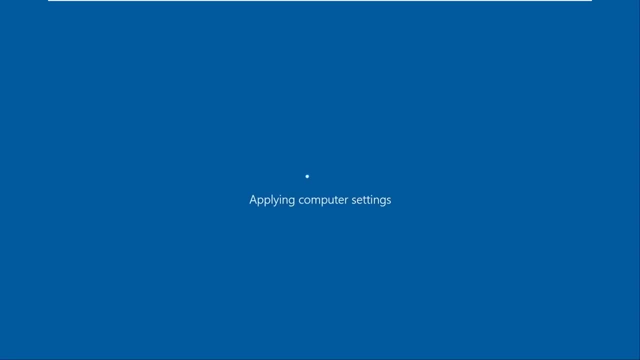 Have I ever been to DEF CON? Yes, I have been to DEF CON. I've been there one time. I am open to going back one more time for somebody to change my opinion on how I felt It could have been the company that I was with. 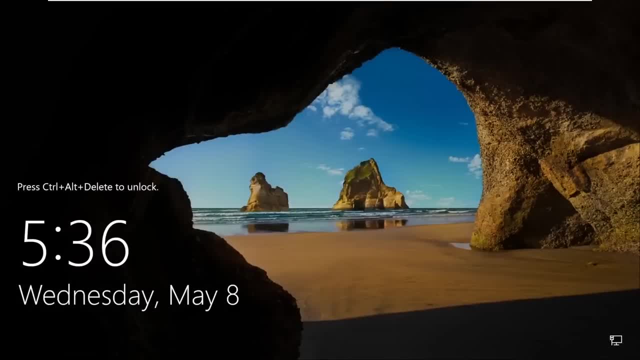 But as far as, As far as it was, I didn't enjoy myself that much. I'll answer a couple more questions. Any tips for security analyst interview? I will get you that after the fact. Ask me that again. I've got links for that. 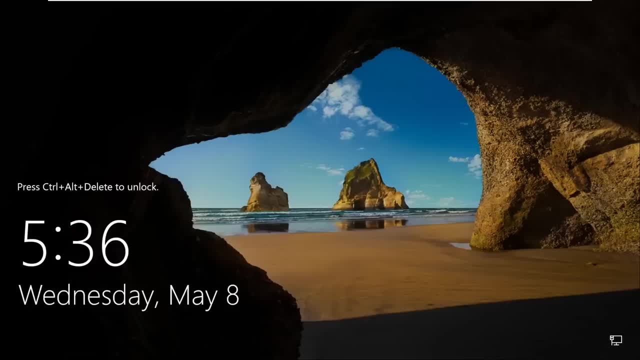 And then we'll talk. And then somebody said: EWPT to ECPPT to OSCP- Is that a good path? Yeah, that's fine. However, you want to do it Solo. I think all of those, I think all of those sorts of things would be a really good way to break into the industry. 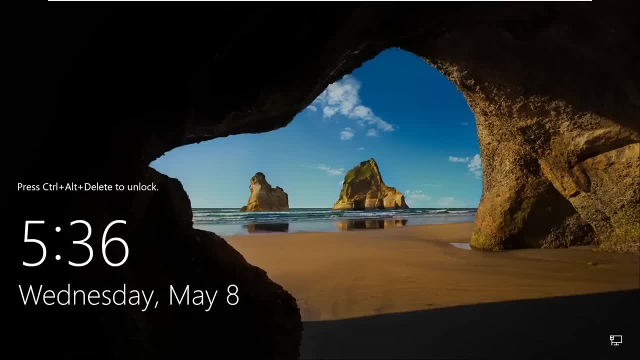 Yeah, you can PM me if we're friends. If not, just add me, Eric, and we'll go from there. I've got links for you, All right, So we are back into this. So let's Alt-Ctrl-Delete with our little three buttons up here. 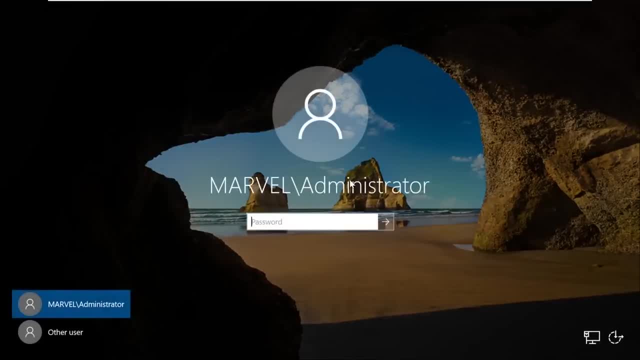 Now you see, All right, So we are back into this. So let's Alt-Ctrl-Delete with our little three buttons up here. Now you see that we are Marvel slash administrator. We are on the domain. I left my caps lock on. 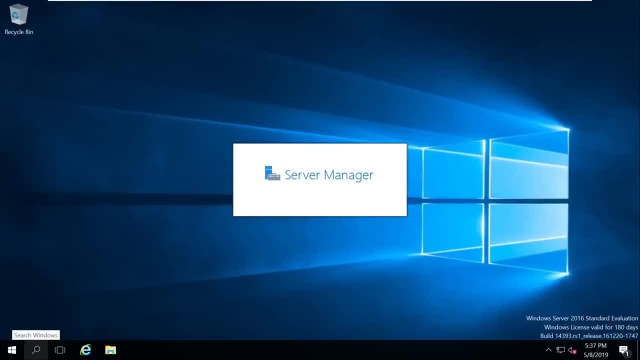 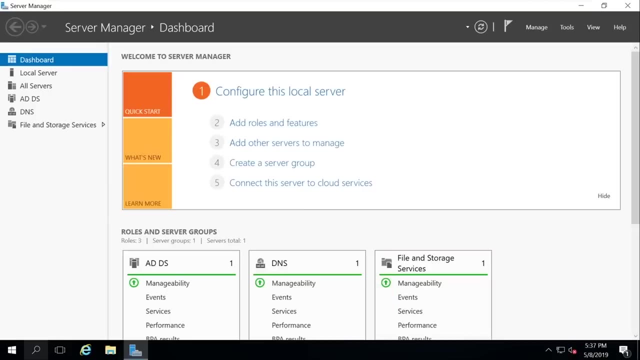 After you promoted the domain controller, you did something. What did you do? So when I hit Promote, you are going to name your root domain. You're going to hit Add a New Forest, Name your root domain. You're going to add a password after that where it says to add the DSRM. 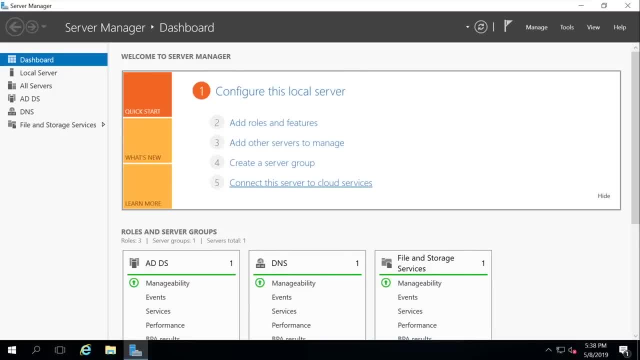 And then you're pretty much going to just next, next, next through all of that and hit install, All right. So now we should be on our domain So we can come into tools in here and we can say: Active Directory Users and Computers click on this. if we click on the forest of marvellocal and you say domain controllers. 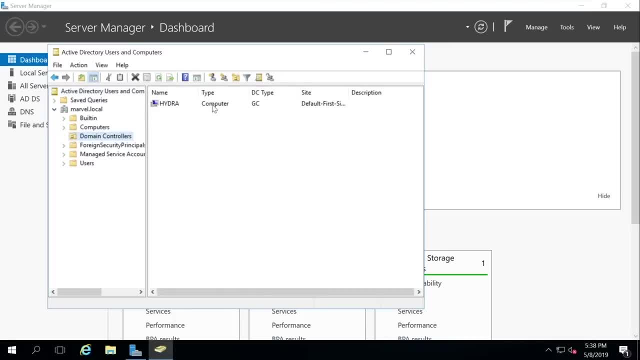 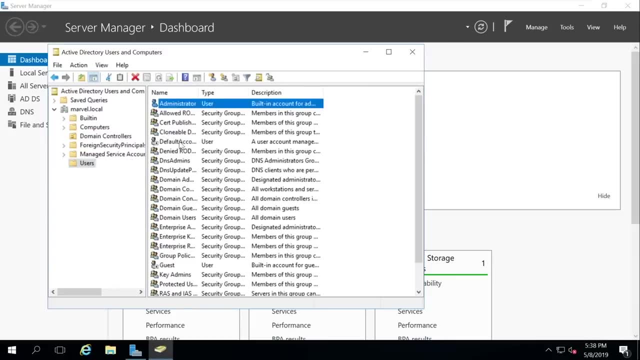 you can see the hydra is now acting as our domain controller. we also have users down here, so we've got an administrator. uh, looks like a default account has been disabled. guest account has been disabled. you can tell by the little logo next to them. uh, so what we'll do is we will. at least i think it's disabled. um, what we'll do is we're going. 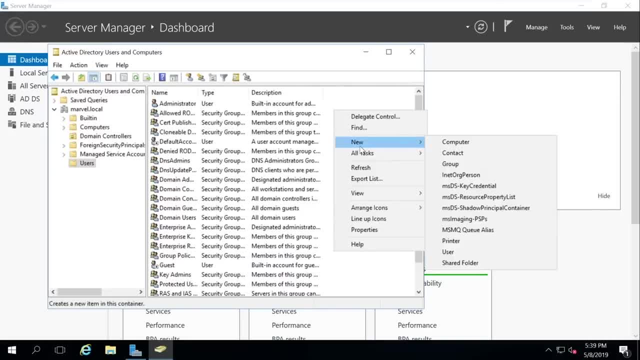 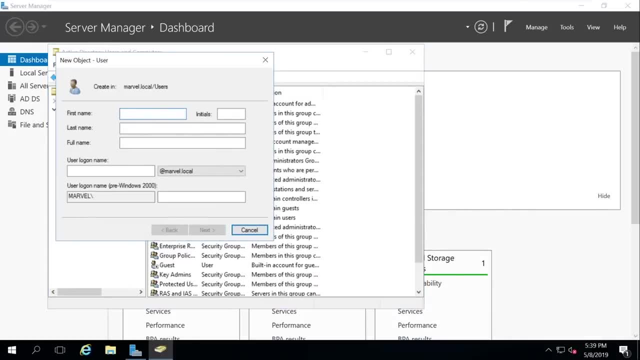 to right click in on this users group. here we're going to say new and we're going to say user. so you guys should know what marvel character i'm a fan of. that is my man, frank castle, and what we're going to do is we're going to say f castle. 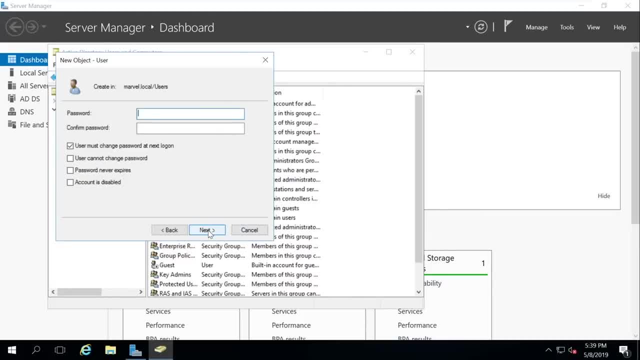 first initial, last name, hit enter. next we have to set a password for him. uh, let's make it something kind of basic. let's also make this password one p-a-s-s-w-o-r-d-1. if it lets us do that, capital p, rest is lowercase, and then a one. 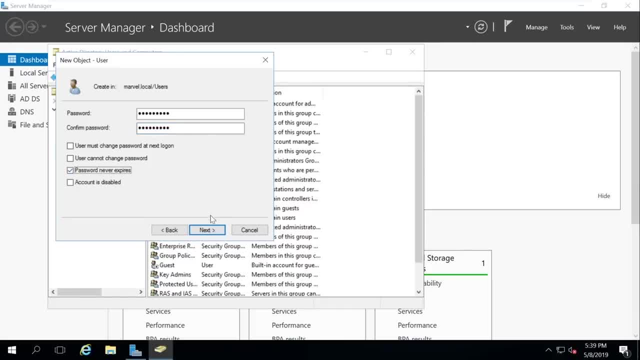 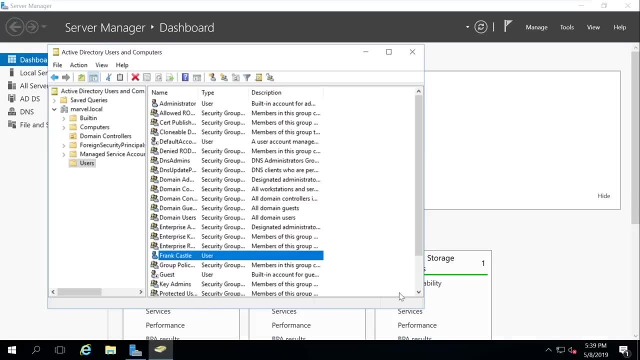 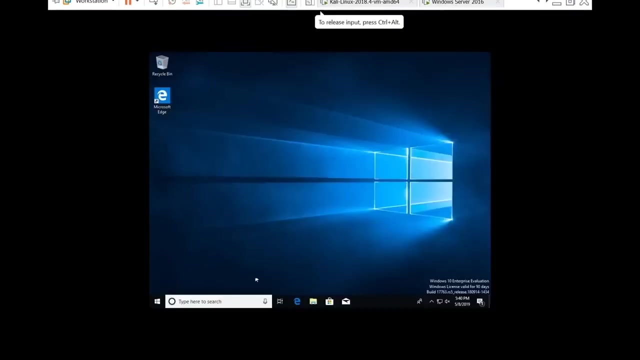 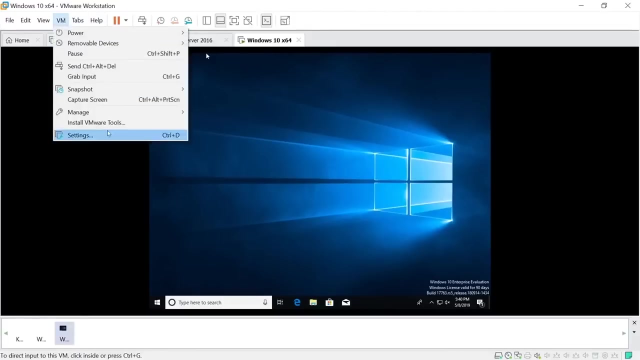 we'll say: password never expires because we're bad admin. finish, techno bro. hey techno bro. how are you doing? man, all right. so we've got frank castle. let's go over to our windows 10 machine and let's install our vmware tools while we're at it, to make this nice and pretty. 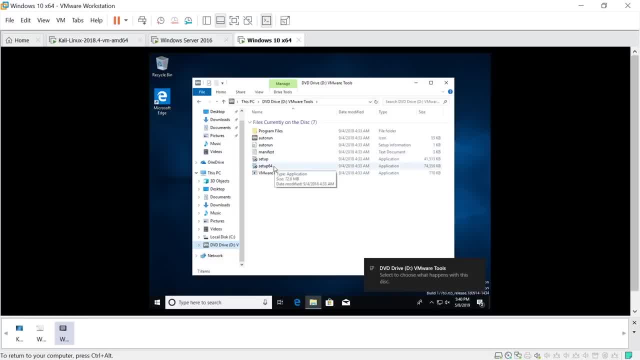 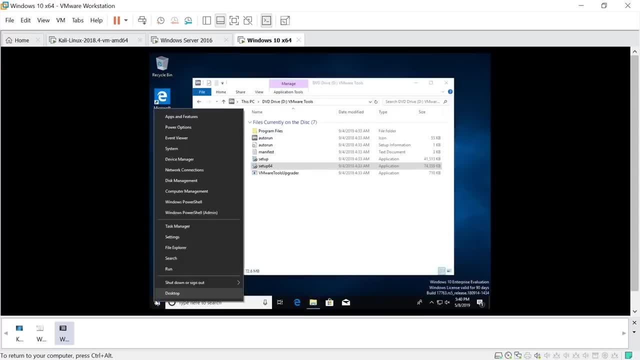 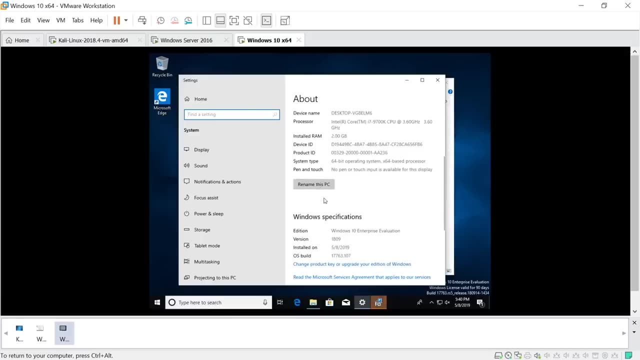 and i think it's a little different. you can't just right click on system to change the. well, i guess you can here so we can rename the pc, um, so i'm going to name this. well, he's the punisher. right, we'll just call it. we'll call it the punisher. 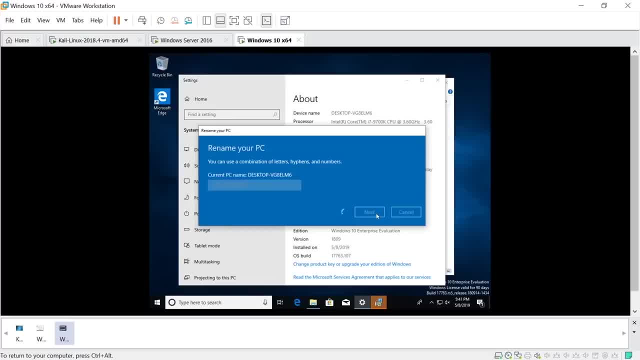 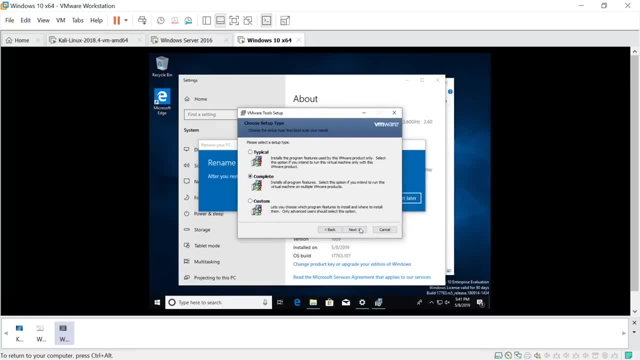 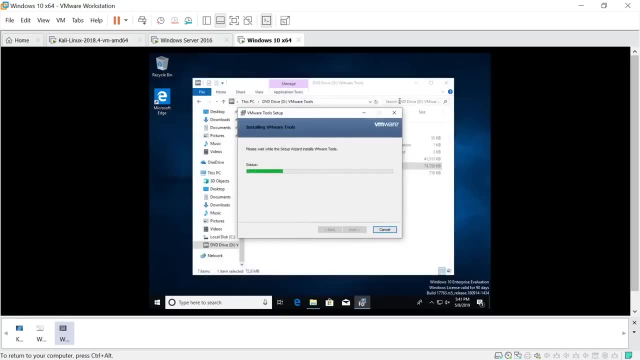 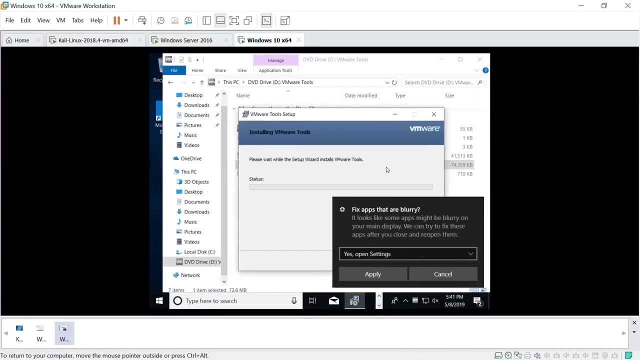 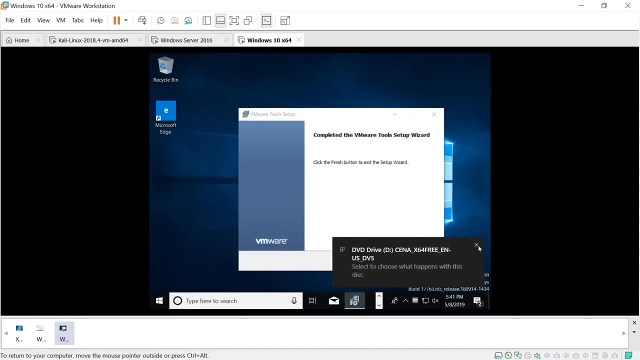 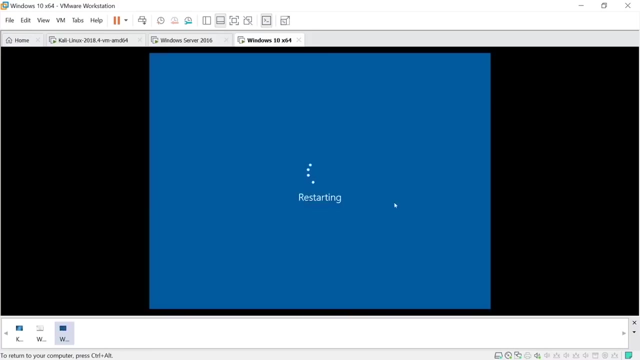 for his pc name and we'll reboot everything. when we have the opportunity to here in a second do a complete install on the vmware tool setup, we'll restart later on this one close out. thank you, techno, i appreciate it. okay, finish and we're going to reboot. should give us a new- uh, a new view on things and a new computer name. 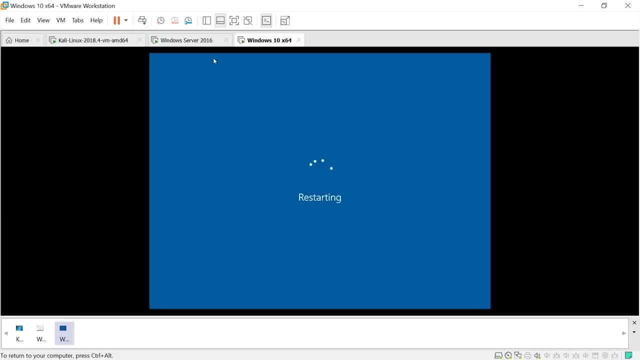 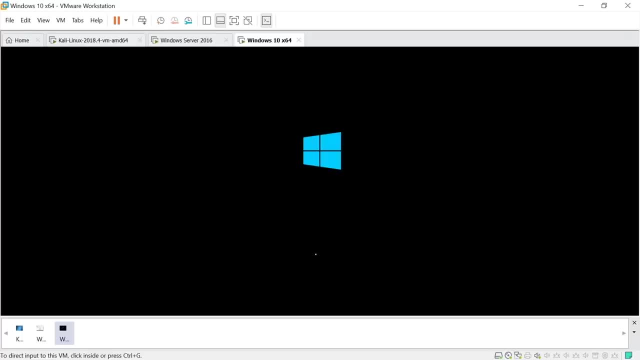 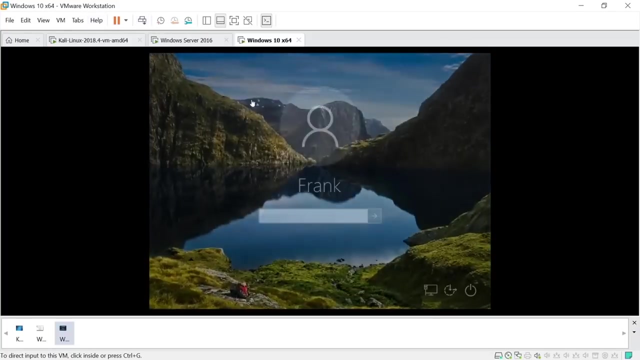 here we go. thought my computer just froze. there it was the mouse stuck on the screen. it wasn't going anywhere, stuck in the vm, but the mouse wasn't moving. so that was fun. all right, let's go ahead and type in frank's insecure password. a password one. 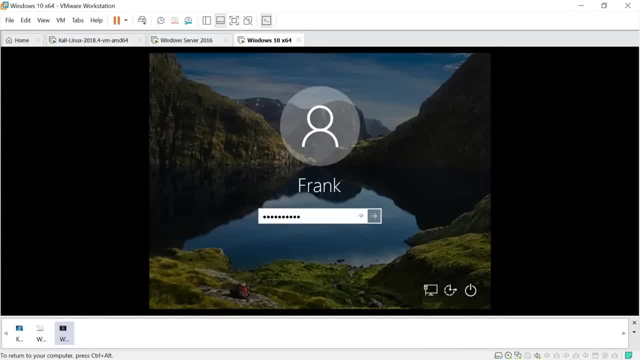 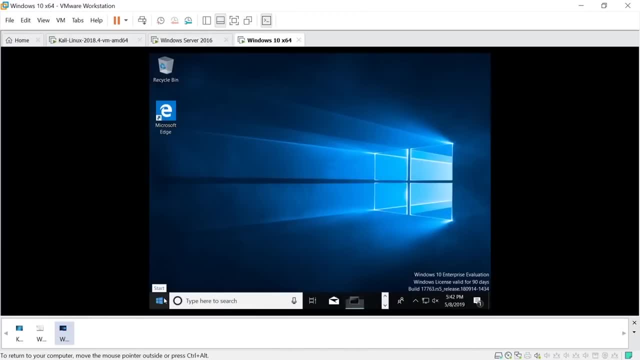 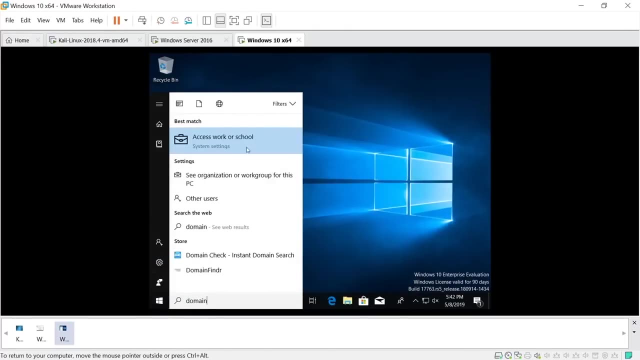 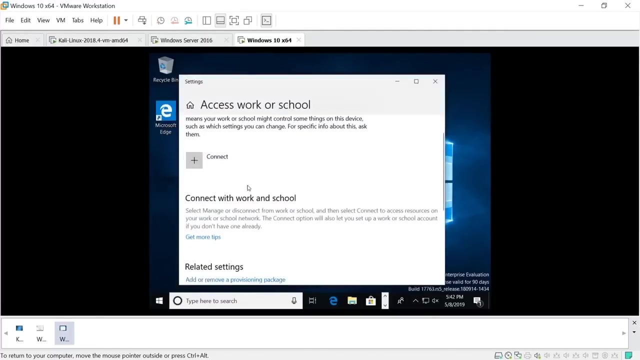 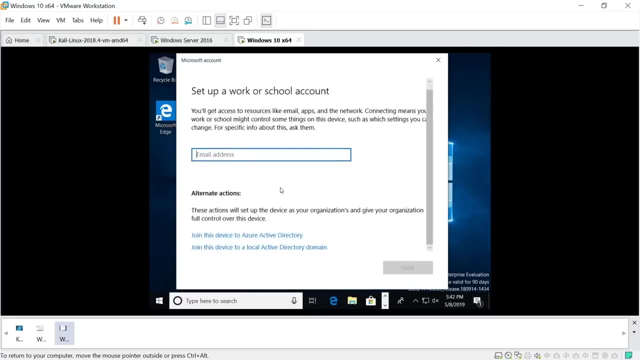 okay, and now we're going to join a domain, which it's a little different. I just type in domain. it says access worker school. I click on that and then we hit connect here, and I don't think this is going to work. join this device to a local active. 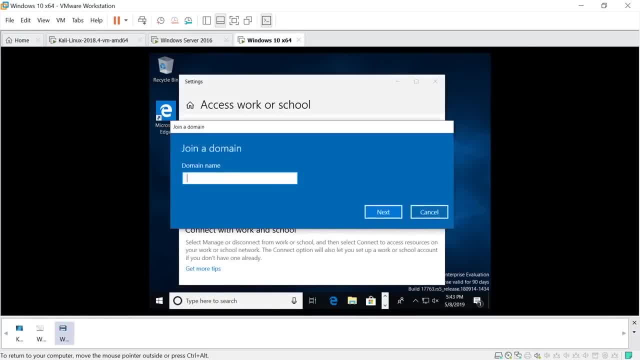 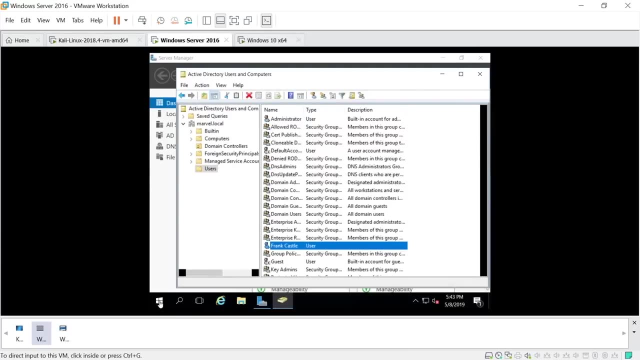 directory domain. I don't believe this is going to work. we're going to try it, though. so we'll say a marvellocal hit next. it's not going to find it okay, so we got to do one other thing in here. so let's go into the server 2016. do command. 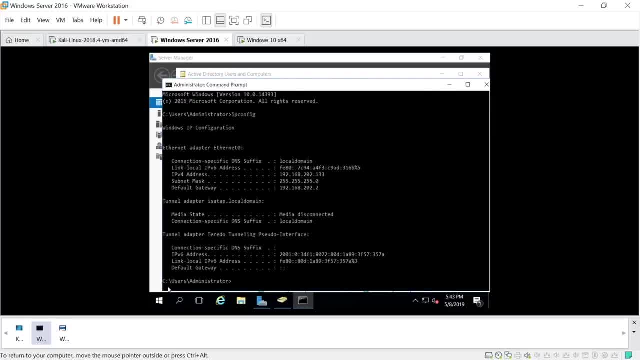 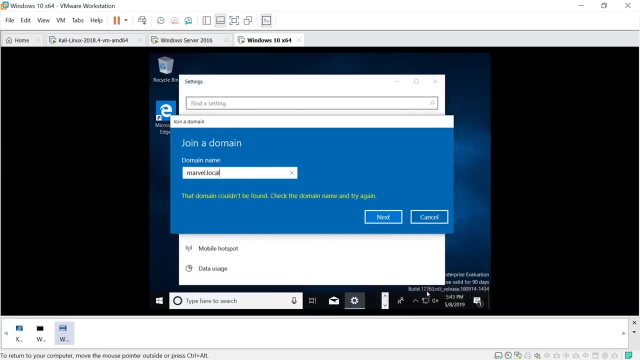 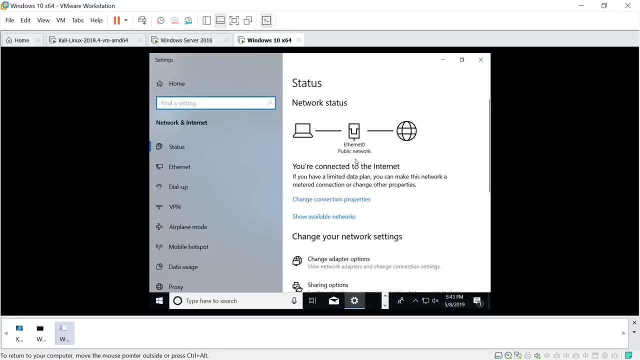 prompt and we're going to say IP config. now my address is 202.133, whatever your address is, just copy this. we're going to go right click on the little internet icon, open your network and internet settings, and that's going to get in the way. we may have to just cancel this. I. 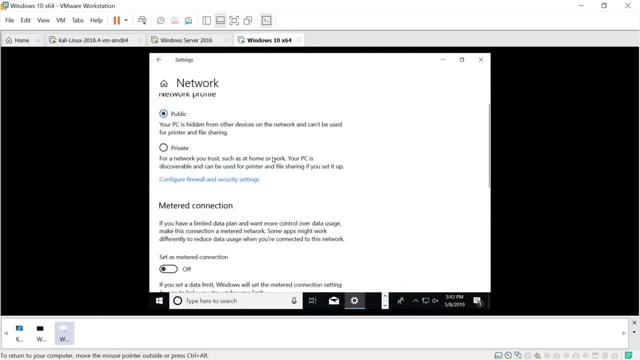 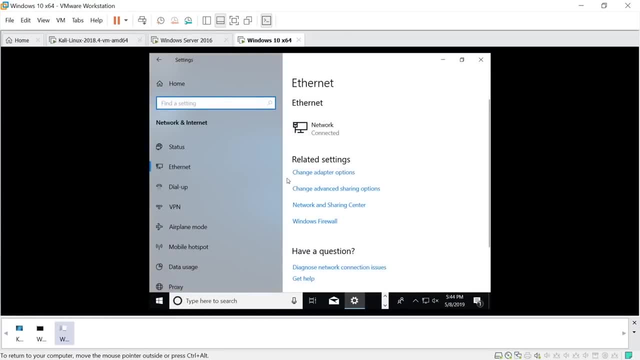 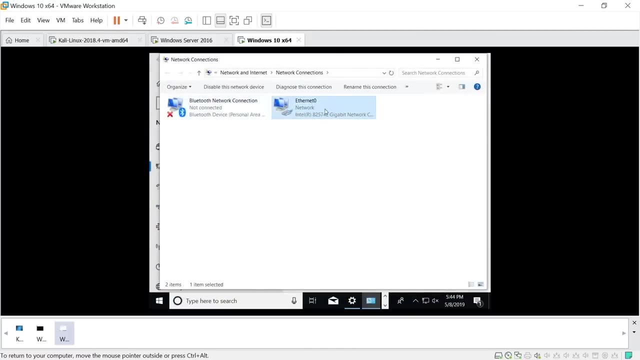 never know how to get there. let's say, change connection properties, and then I think I hit back and it just takes me there. yeah, that's how I know it used to be an easy right-click. go to adapter settings, change adapter options right here, and then you come to this Ethernet 0. you right-click, you say: 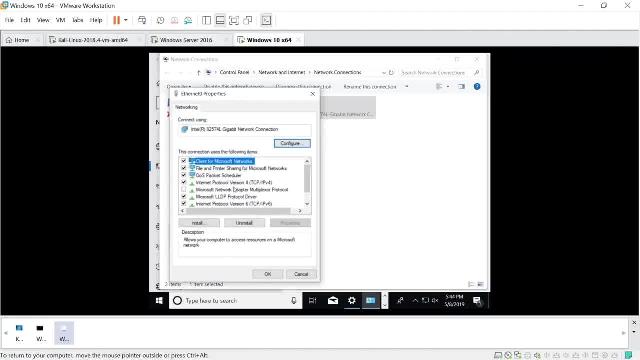 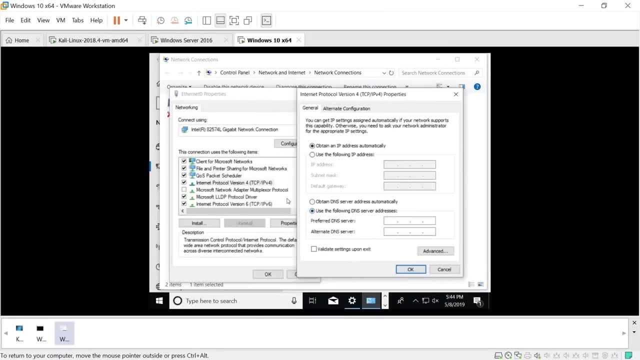 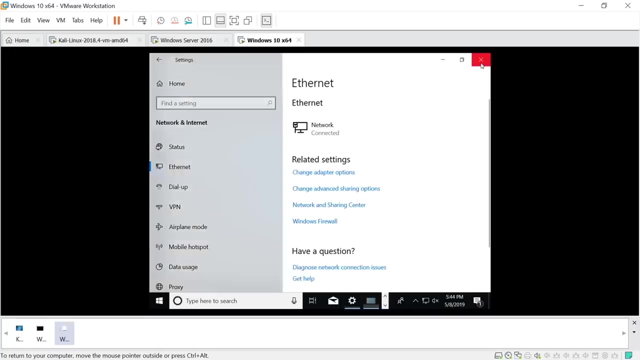 properties. go to IP v4, double click on it and we're going to use a DNS server again. IP address is 202.133 for me. well, you, I'll do the old 8.8.8.8 on here. hit, okay. okay, it may or may not work, we may. 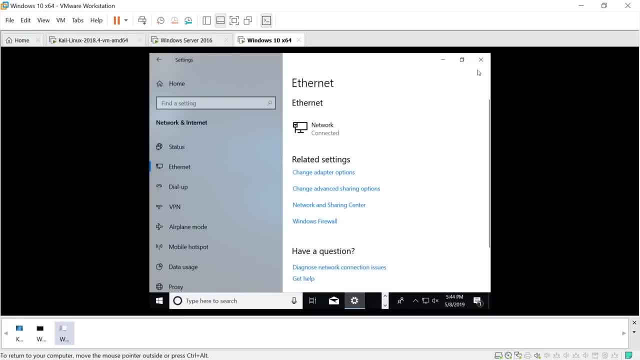 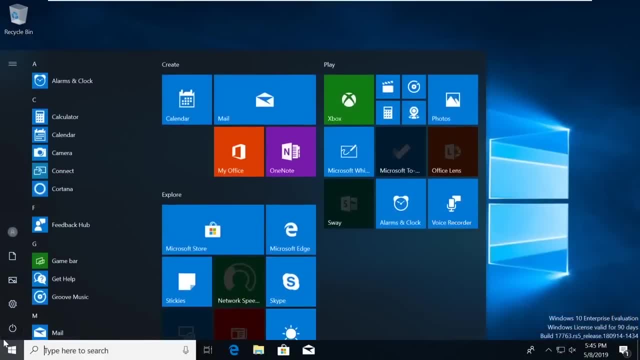 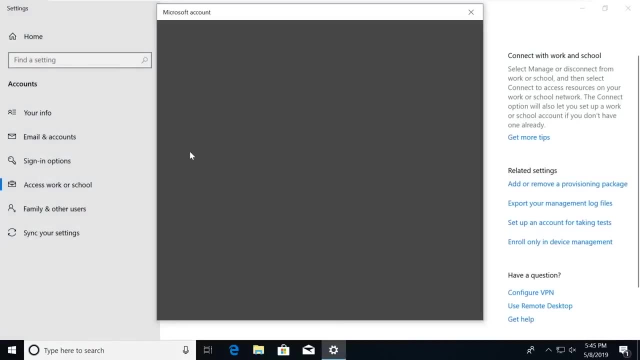 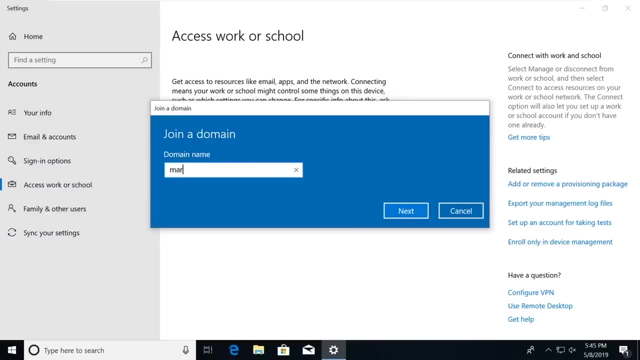 have to flush the DNS. close out of that. actually, let's see if we can full screen. there we go and we're gonna say domain again: access, work or school. hey, connect you, join this device to a local active directory domain. let's try this one more time. 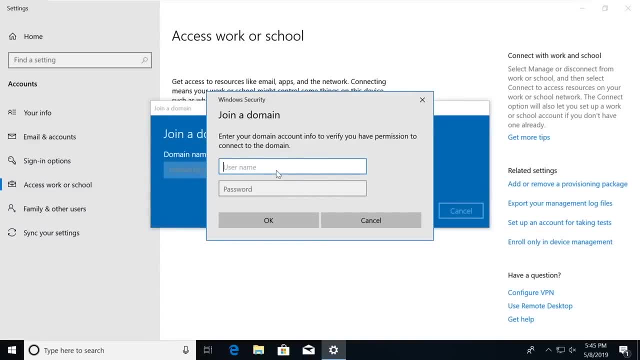 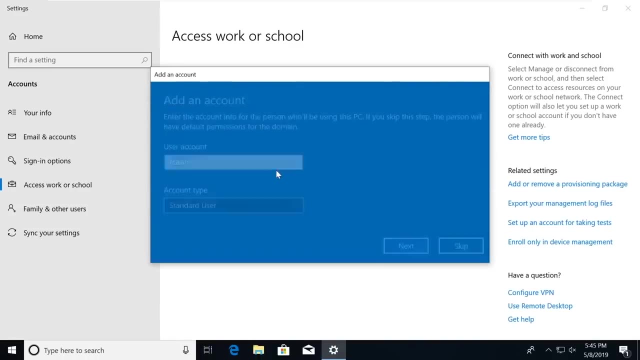 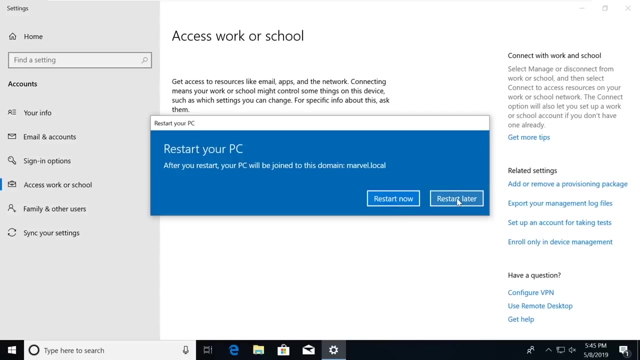 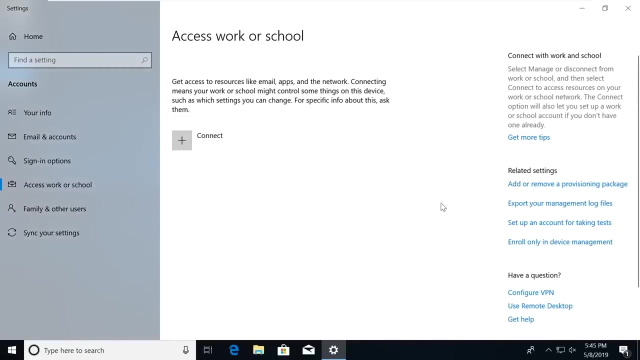 there you go. so now we get the pop-up. so our user is fcastle, our domain is going, or our password is password. one hit, okay, so he's gonna be a standard user. hit next and we're gonna restart. somebody said one dot, one dot, one dot, one, true. somebody said control net connections. 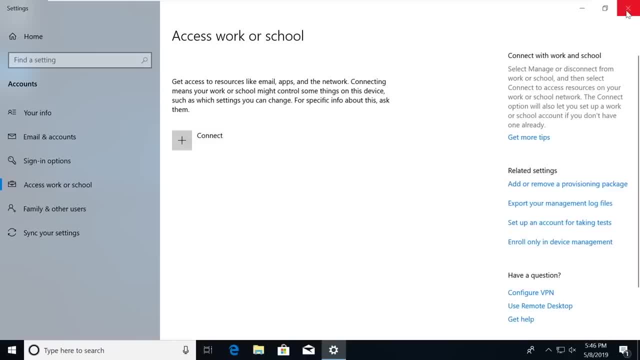 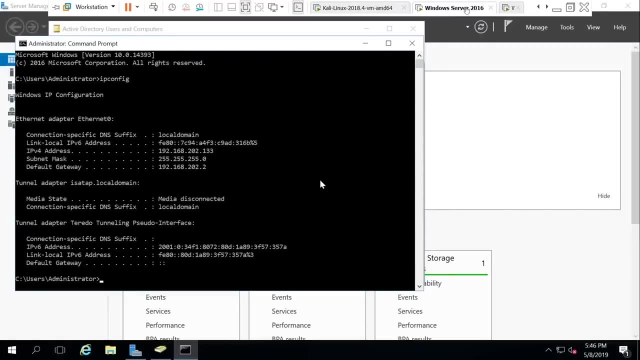 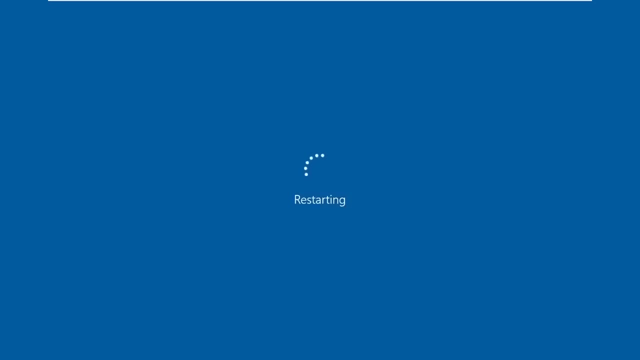 from command is a shortcut. I've never used that one. I'll have to try that. so this should start rebooting. if it's nice, let's just give it a nudge, and when we come back we should have Marvel and Frank Castle, meaning that we have officially. 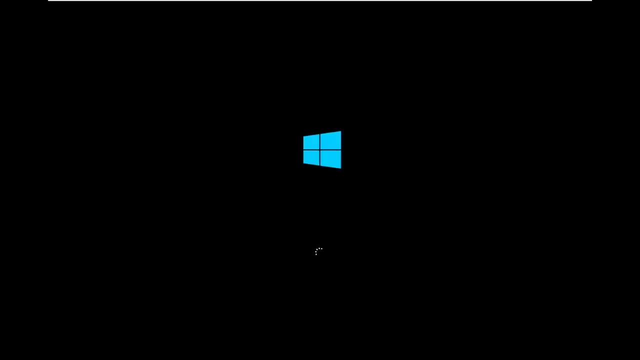 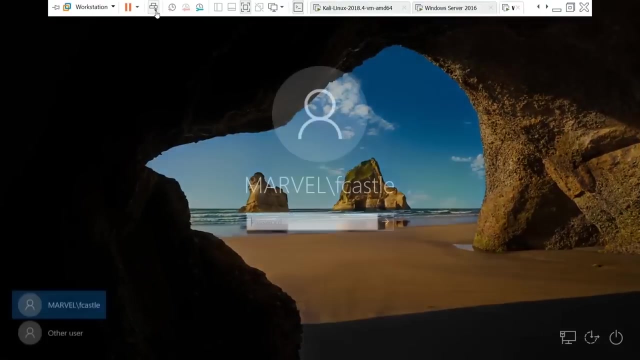 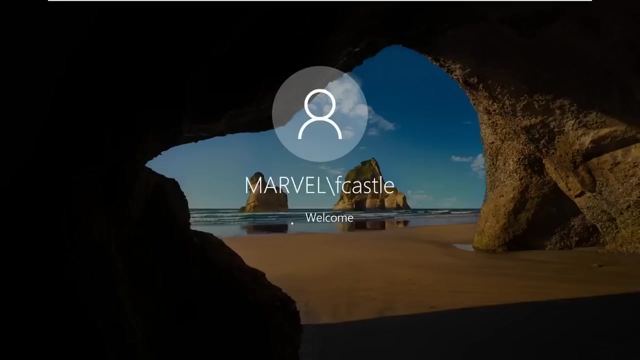 joined the domain, we are on our active directory environment and now we can start doing some malicious things. let's make sure that that is true. I'll give you guys a minute to catch up as well. okay, again, Marvel fcastle, let's go ahead and log in. good old Frank's logging in, he's gonna have. 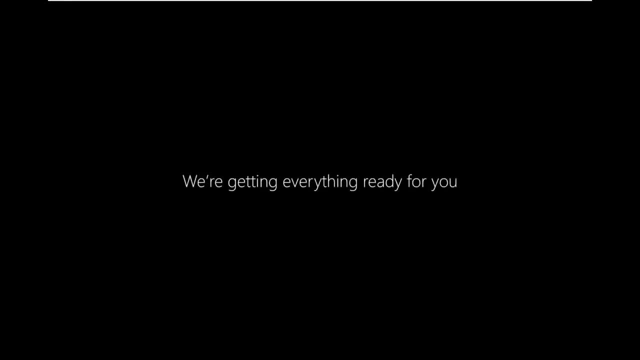 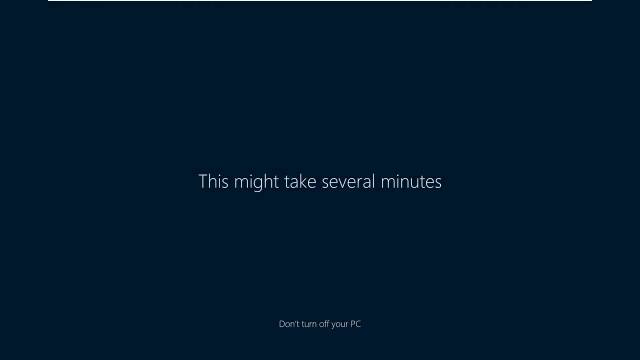 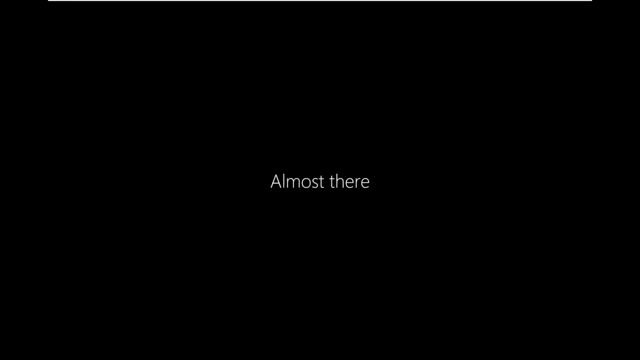 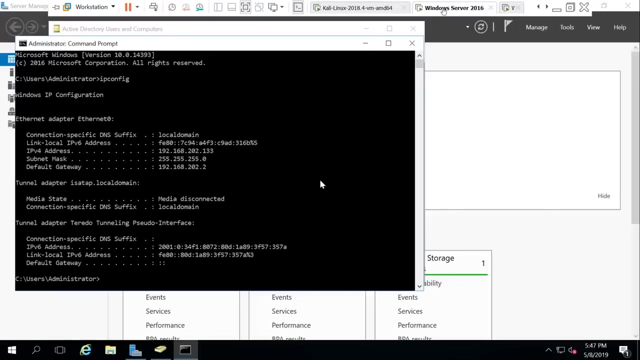 this profile built for the first time. we've all seen this screen too many times in our lives, I'm sure. all right, well, this is going, let's go ahead and go back over to Windows Server 2016, and what we're going to do is we're going to create our first scenario, and this is going to be one of the things. 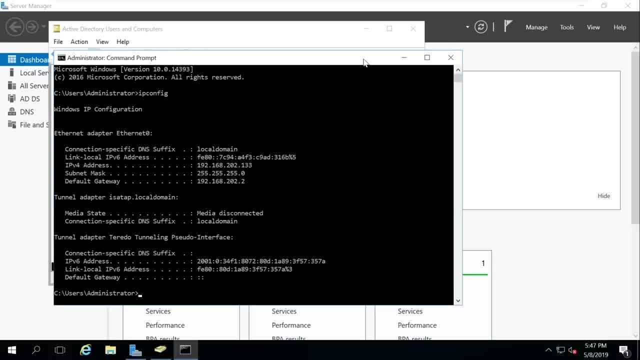 we focus on a lot in this, in this lesson over the next coming weeks, is we're going to be focusing on the first scenario and we're going to be focusing on the first scenario and we're focusing on SMB, because SMB is one of the most exploitable things that we're going to have. 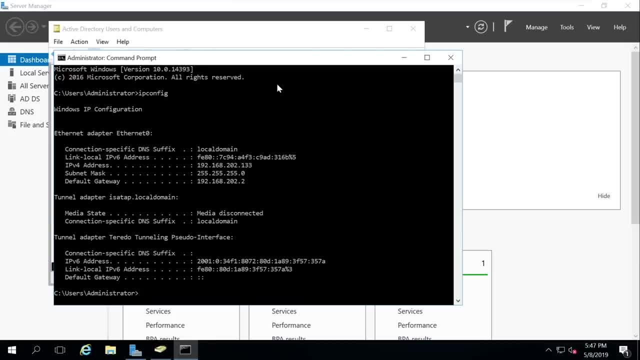 Now for LLMNR poisoning. it doesn't have to be SMB. We're going to get into what exactly it is here in a second And we'll talk about some techniques that I've used on pen tests that are kind of outside the box Something to think about. So let's close out of this. 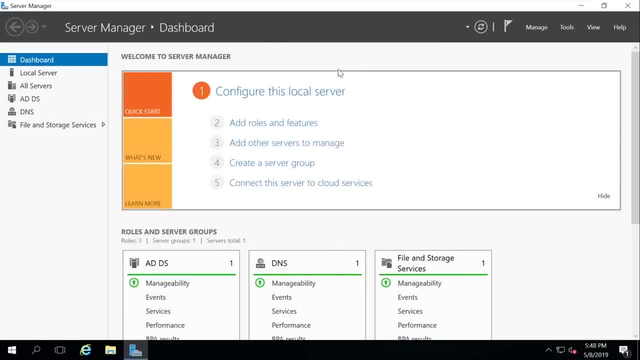 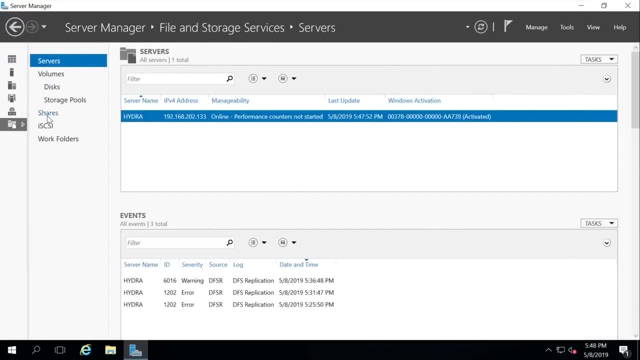 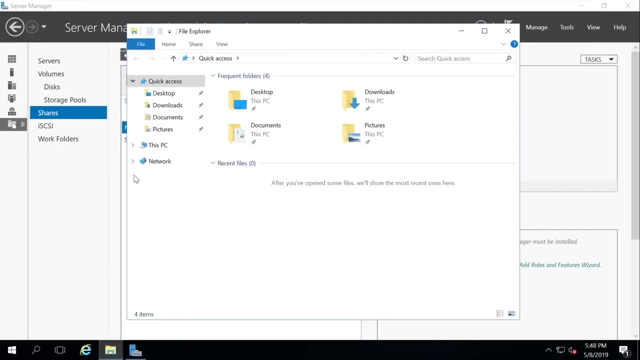 close out of this. So in your server manager you're going to come over to file and storage services. Over here we're going to say shares And what we're going to do is we're going to open up a new folder here. Let's go to this PC, Let's go to the C drive And we're going to right click. 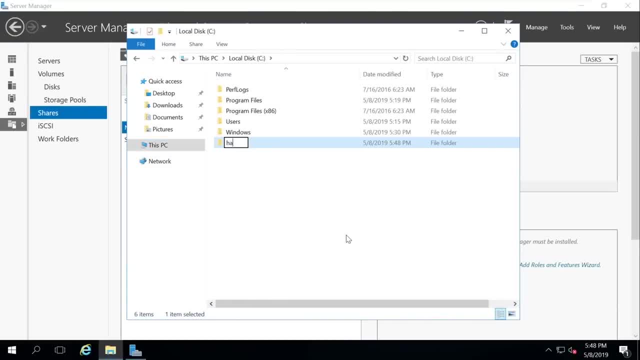 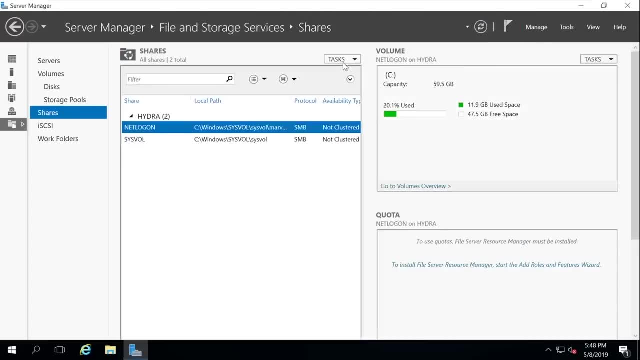 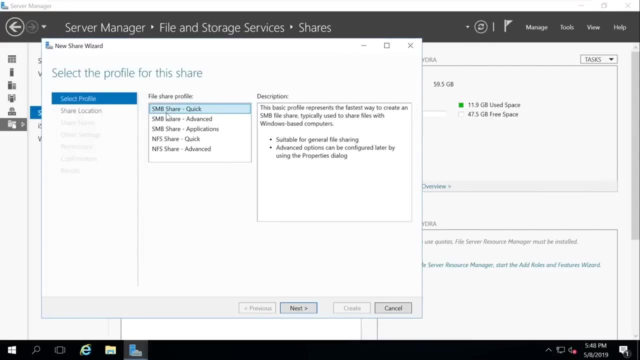 and make a new folder. We're just going to call this folder: hack me, Okay. So we're going to create a task up here Under shares. we're just going to say new share. It's going to be an SMB share, quick. 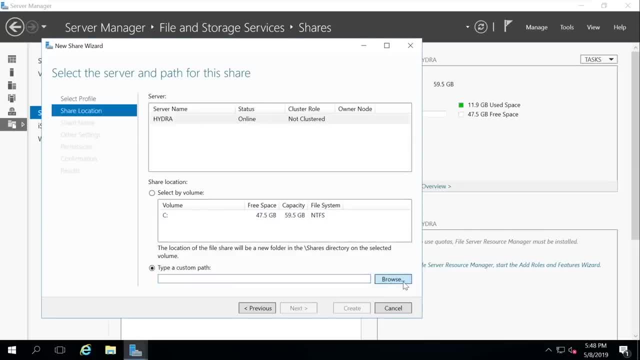 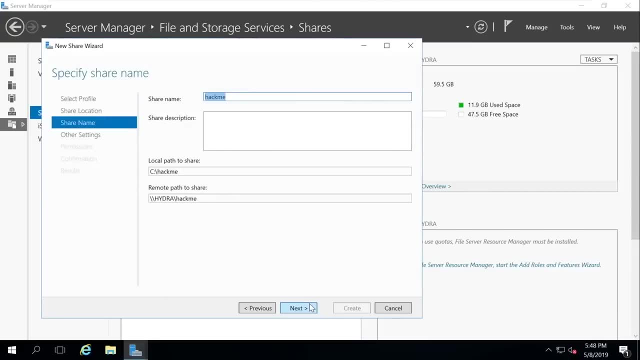 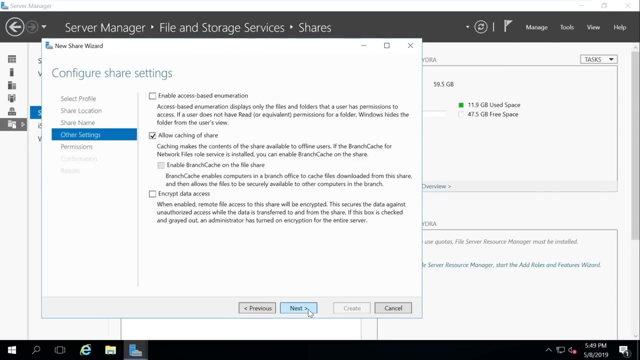 We're going to select the share location under custom path And we're going to select that hack me folder. Hit next Share name is hack me, Hydra. hack me will be the path to the share. Allow access based enumeration displays only the files and folders that a user has permission. 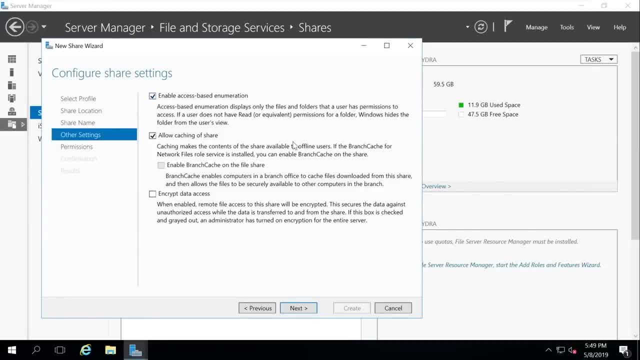 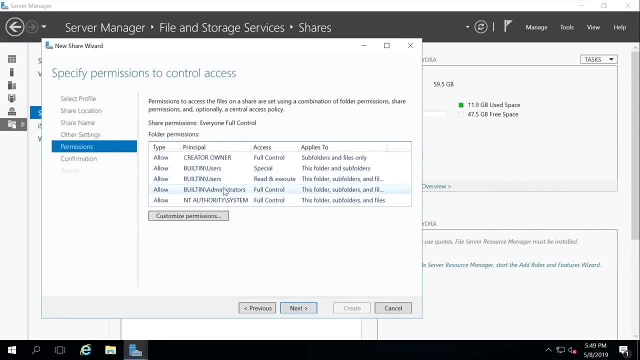 to access. So if the user doesn't have permission, let's go ahead and set that We're not going to encrypt it. I'm just going to hit next. Hit next. You can see that it's doing the. if we go into 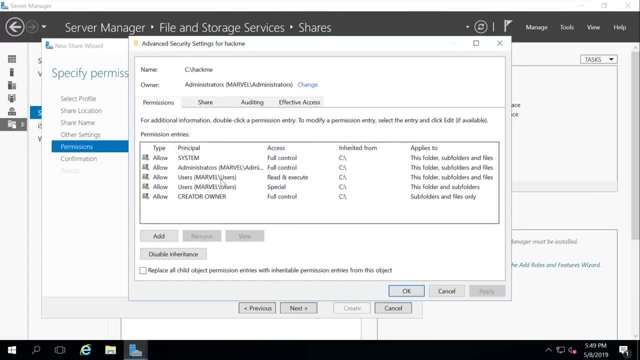 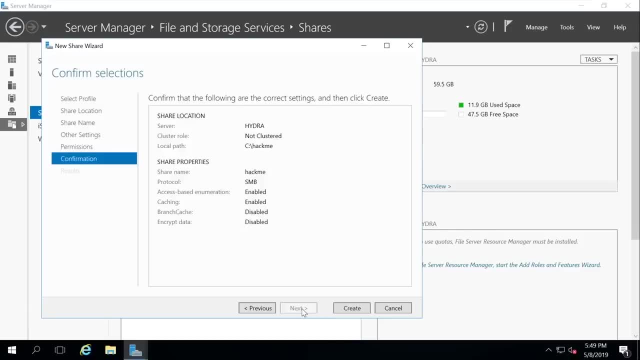 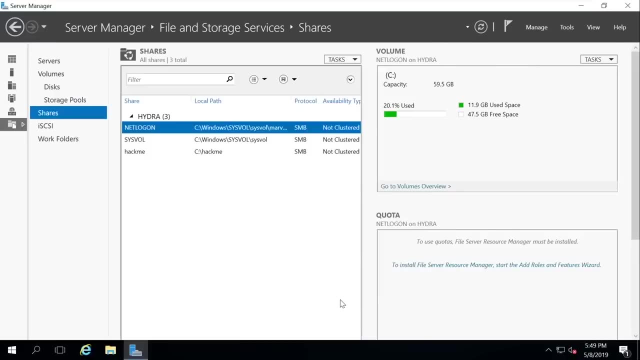 customized permissions. you can see that it has administrators and Marvel users have read and execute status. So we'll hit okay, Hit next Share And we're going to hit create And it created it just like that. So we go back and we go back. 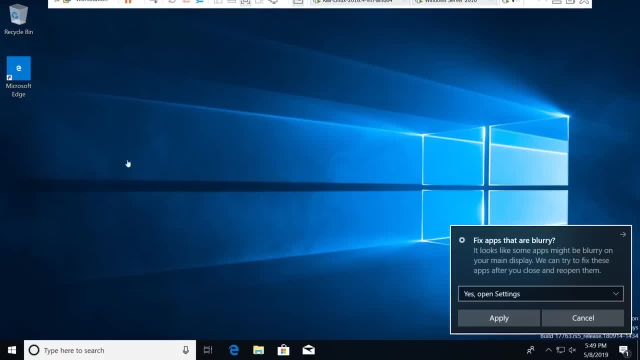 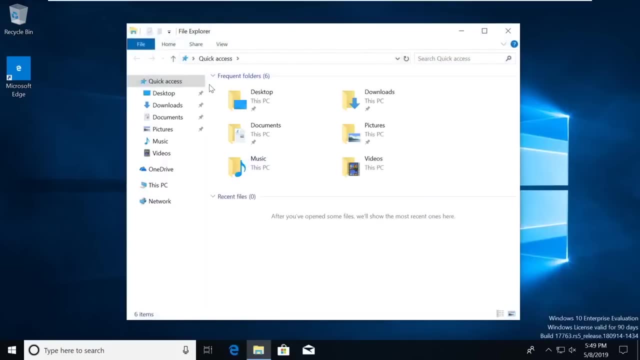 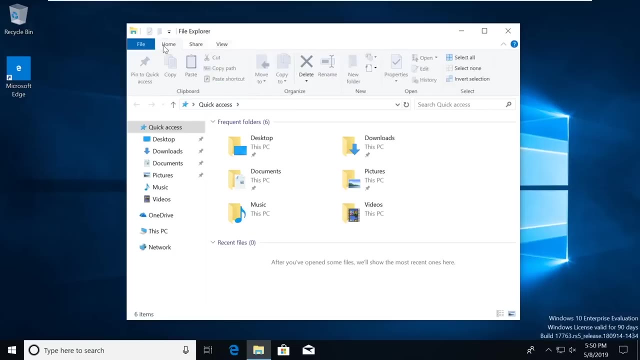 over to our windows machine. We're going to add that share, So just go to our folder. If you go into, where's the button? Maybe I need to be this PC. There we go. We click on this PC. You say map a. 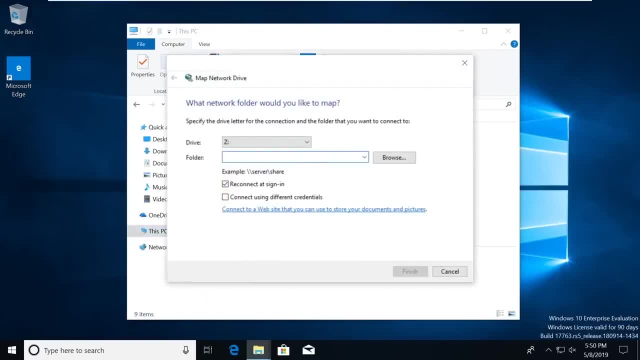 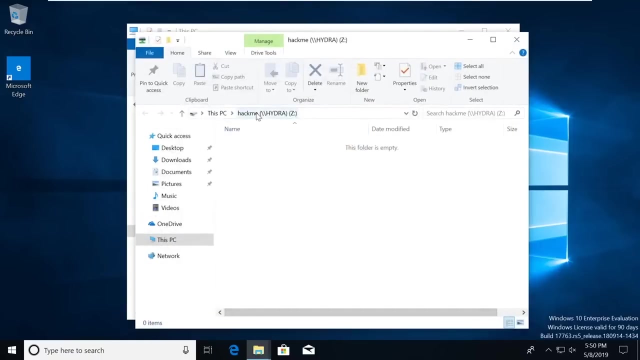 network drive. We'll just call it Z drive. You can put it whatever drive you want. Say Hydra Clue. Oh, you can do it either way. Okay, Reconnected. Sign in, Hit, finish And now we have access to this Hydra hack me folder. 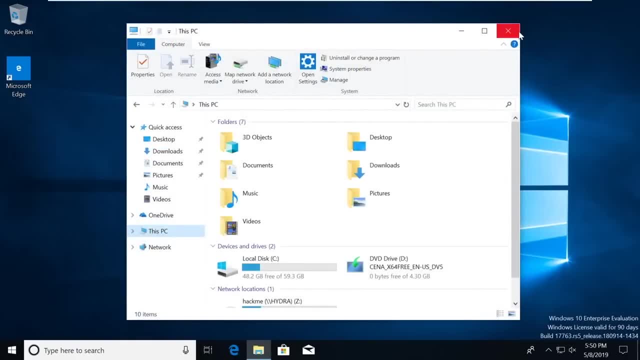 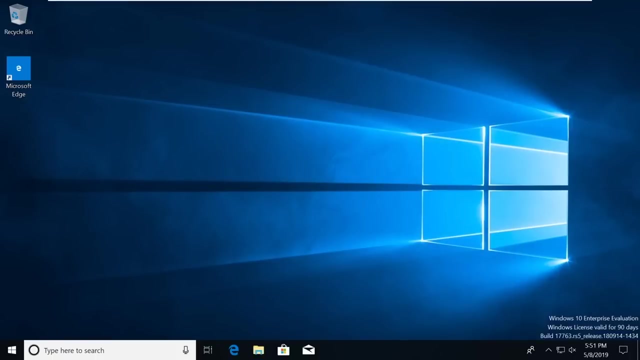 Our lab setup is complete. Give me one second. I'm going to drink some water and then we're going to go on to a little bit of exploitation and then wrap it up for the night, All right. So what we're going to be talking about tonight is LLMNR poisoning, or also known as 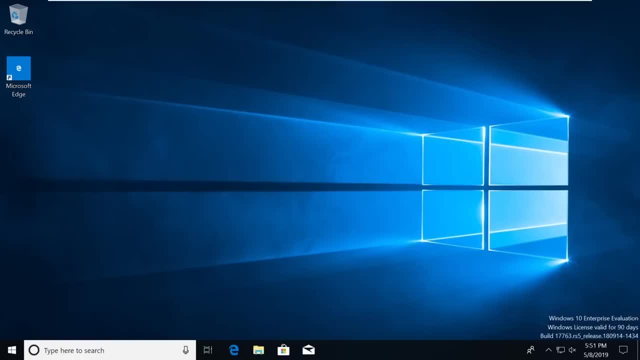 NBTNS poisoning. So your LLMNR, that's your link- local multicast name resolution. Your NBTNS is a little bit older, but that is your NetBios name service. So basically what they're used to do is they are used to identify hosts when the DNS fails. 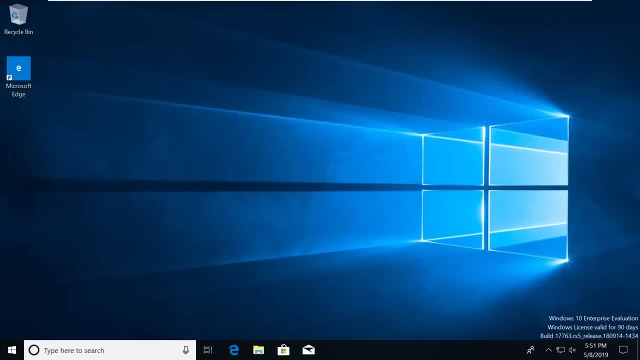 And a big flaw of LLMNR and NBTNS is that both the services utilize a user's username and their hash, their Windows password hash, typically NTLM V2, sometimes NTLM V1. So when it gets responded to it sends over a hash And we're going to take a look at what that might look like in a man in. 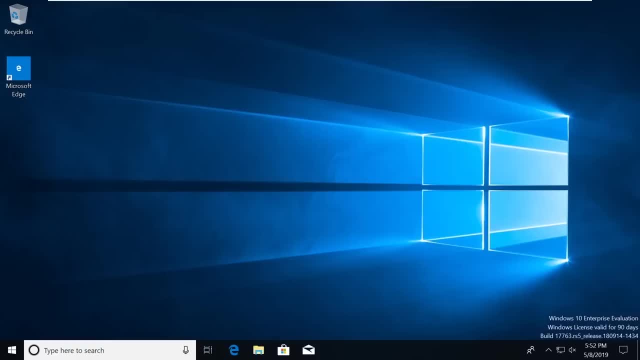 the middle situation here. in a second I've got a little nice little info Graphic, But also it's just a way to you know, connect to like a share, just like we're doing now using this name resolution. So what we do as an attacker- and let me pull this up- 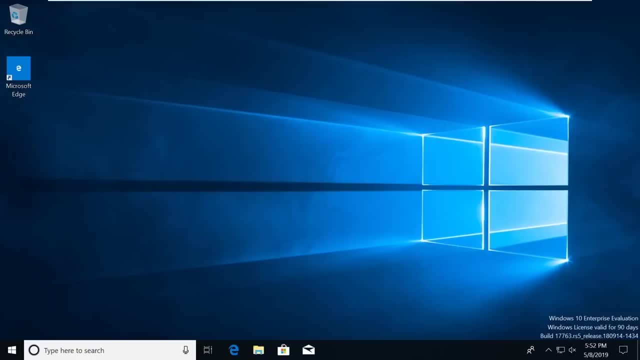 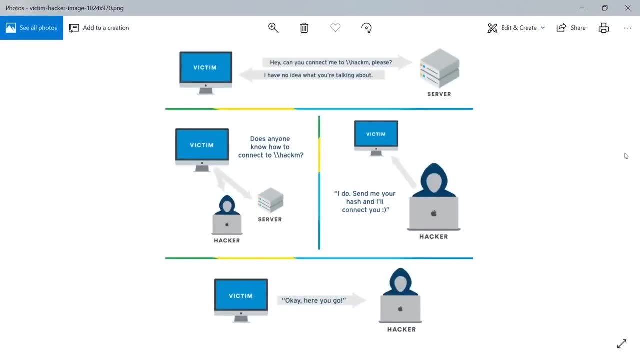 Somebody said: repeater, you're close, It's responder. But what we do as an attacker is got this nice little graphic here. So this is a classic man in the middle attack. What's going on is across the network, there's all this traffic back and forth and these hashes are flying back and forth. 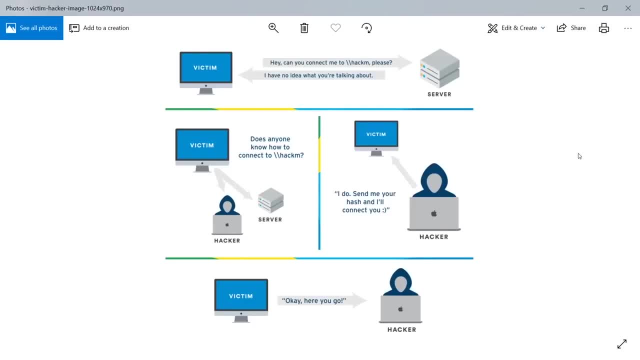 And sometimes there is a mistake or something that generates or triggers this action, right? So what happens is when these hashes go out, typically they're going out to a known share or known device. Sometimes, however, they don't know where to go or there's a mistake that happens, And if you're sitting in the man in 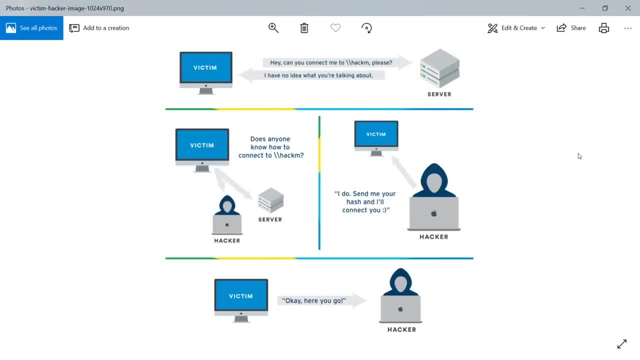 the middle you can say: hey, you send it to me when there's a broadcast message And let's take a look at how this looks. So, for example, there's a share out there, right that we say okay. 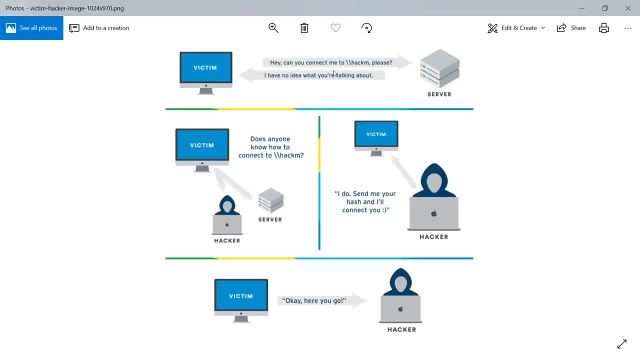 it's going to be hack me right, And we just created hack me But this says: hey, can you connect me to hack M? We typed in the wrong share name. Well, the server is not going to know What the share name is right. It's never heard of hack M before It's heard of hack me. 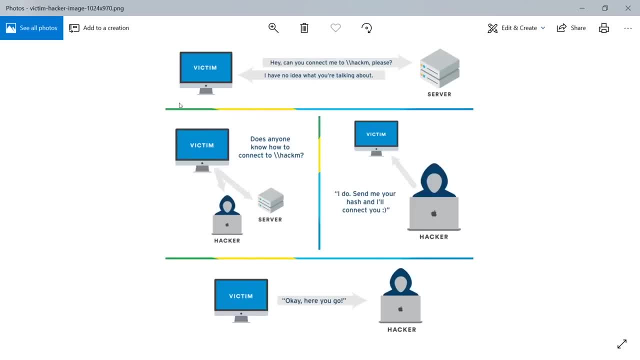 So if it doesn't know what the heck you're talking about, the victim's going to say okay. well, if the server doesn't know, then does anybody know? So now we're going to send out a broadcast message with our hash. Well, not with our hash yet, Sorry, We're going to send a. 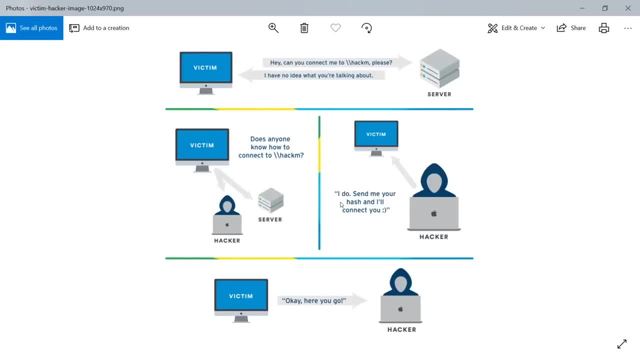 broadcast message: Does anybody know how to connect to this hack M? And me as a hacker sitting in the middle is going to say: I do. I don't know what hack M is, but I'm going to lie to you And I'm going to say: I know what it is, Just send me. 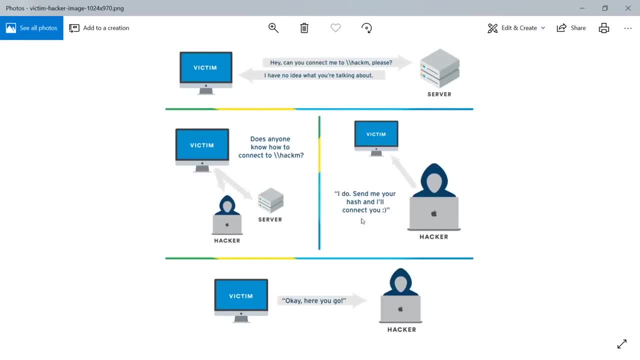 your hash and I will connect you to that hack M folder, And the victim's computer is just going to say: okay, here's my hash, So this becomes dangerous, right? There's a couple of different attacks And we're only going to talk about one attack today. We'll talk about the second attack. 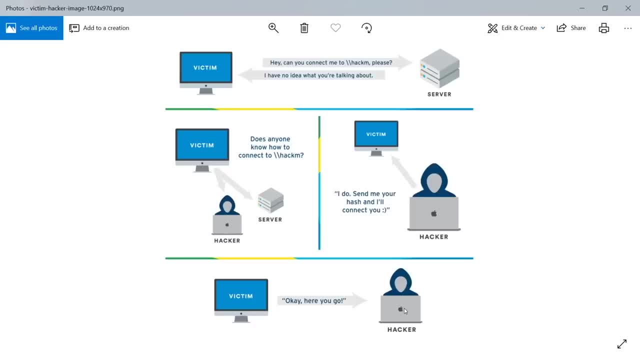 first beginning of next week. So attack number one is: we take that hash, we run hashcat against it and we try to crack the password. If the password is not complex or long, then we're probably cracking it pretty fast. We're. 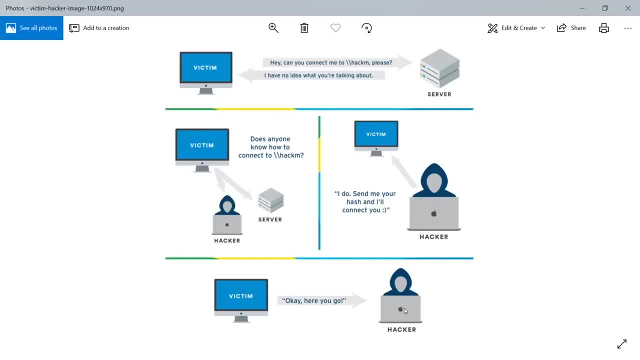 using that to navigate around the network and see what sticks, And we'll talk about those techniques as well Tonight. what we're going to be doing is learning how to capture the password and also how to crack the password, So we'll be doing that. Another idea, though, is, instead of taking that hash, 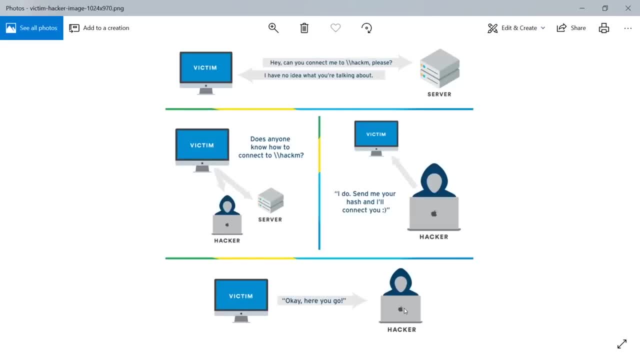 and cracking it offline. another thought is: we're going to take that hash and crack it offline. You can take that and do something called relaying and try to send it to a server and use the hash to authenticate to a server via SMB without ever knowing what the password of that. 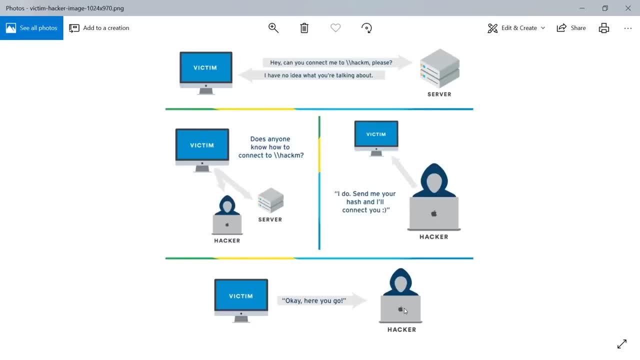 account is. So that's called NTLM relay And we'll cover that next week. So, in order to do what we're going to be doing is we're going to set up a man in the middle, listener with a tool called responder. Now, if you have been following me since week one, in week one we uninstalled 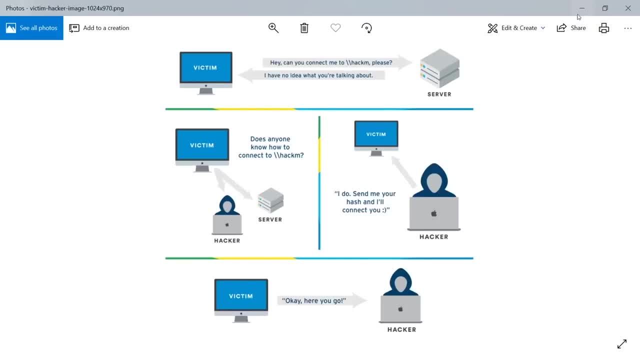 Impact It and installed our own version of Impact It. So if you're all caught up, this should work just fine. If you're not caught up, this might not work. You may have to purge Impact It. We're not going to go back that way. If you just go watch week one video and catch back up, 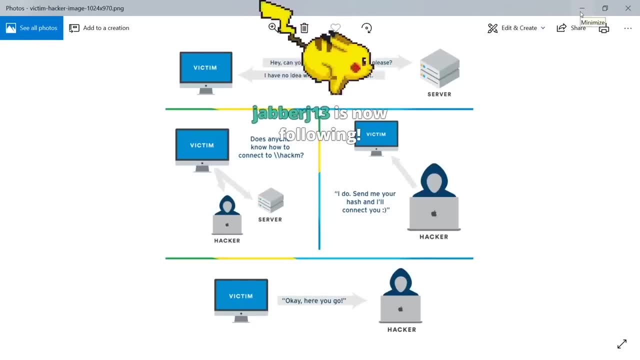 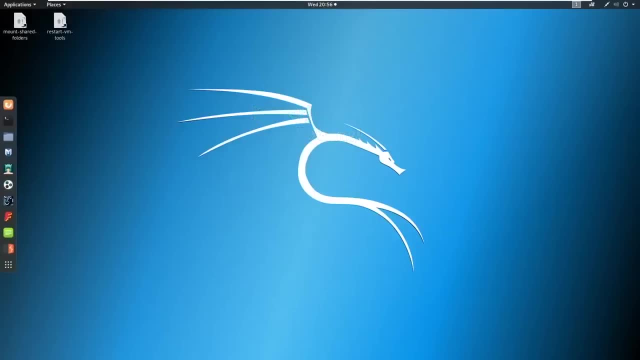 please do so. So let's go ahead and minimize this, And we're going to go into our Kali machine. I'm going to show you how to set this up, And I'm going to talk about how to set this up, And I'm going to talk about strategy here too. So let's just open up a terminal. Let's make this. 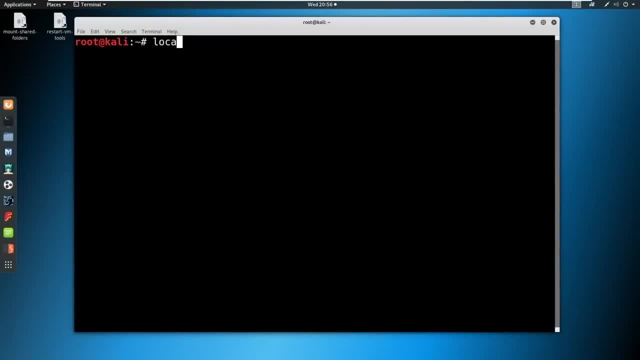 bigger for you guys And we're going to say: locate capital R on this responderpy. Okay, so it should be in your user share responder folder, So let's just cd to that, All right. So what we typically do is, first thing- and this is a scenario we didn't cover- Let's talk about 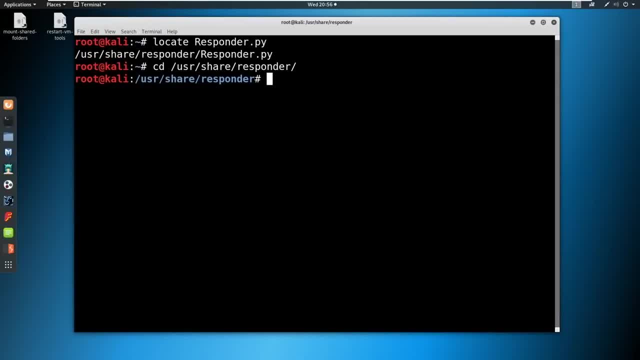 the scenario of what we're in with our network right now. The scenario is: last week we exploited a machine and we got onto the network. We were inside the network doing internal commands. Well, let's say now that we are continuing on from that point, We're on the network, We're. 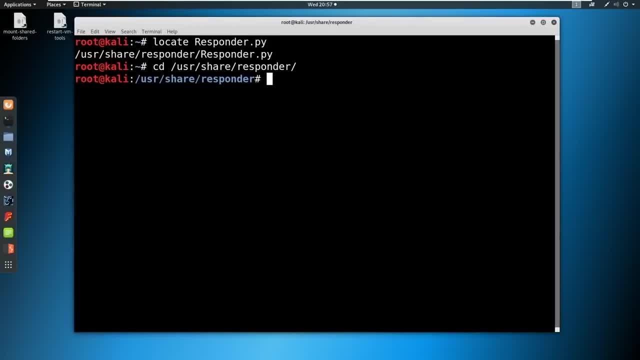 via VPN, Or let's even say that we gain physical access. We plugged in the machine unknown to anybody else and just walked away. So we have remote access to this machine and we're just sitting on their network. No privilege at all, right Just? 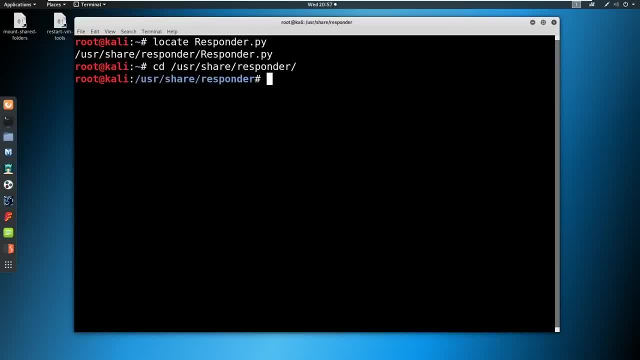 our own rogue computer. So we're going to take this rogue computer and we're going to try to escalate privileges in a way that I would in a penetration test. So the very, very, very first thing I do before I run scans, before I do anything, I turn on responder. 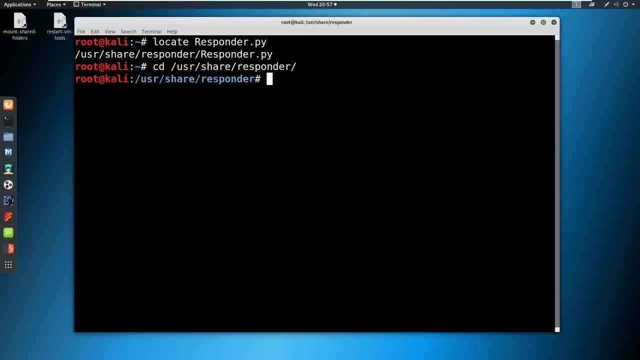 And because the scans- Nmap, Nessus, whatever you run- what that does is that that starts generating traffic. Those scans generate traffic And what responder is listening for is traffic. So if there's a lot of traffic going across the network, the better it is for. 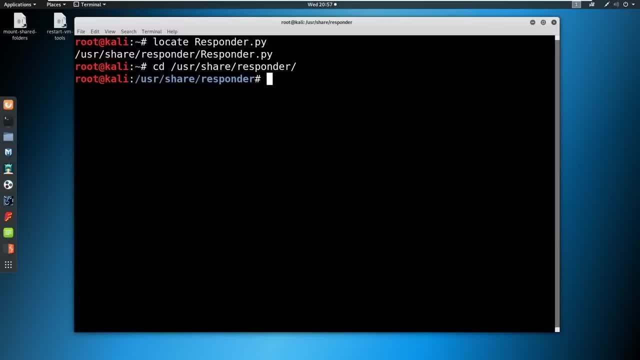 you because maybe something screws up, sends a hash your way and you just gain all the hashes. right, That's the end goal. Now, the best time to run a network is when you have a hash. The best time to run responder is typically in the morning when everybody's coming into work. 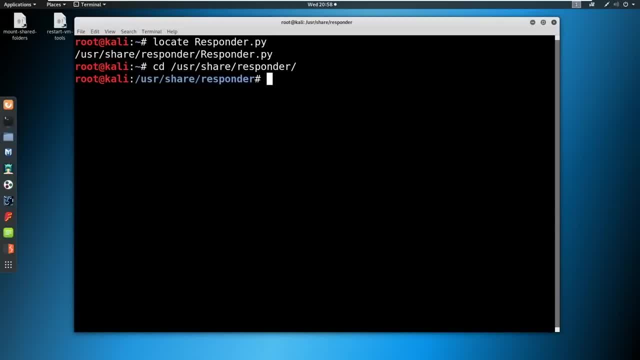 or when everybody's getting back from lunch around one o'clock, So those are your two best target times. You can let it run all day and see what it captures- And typically I do- But definitely if you're doing an internal penetration test, you want to get the sucker. 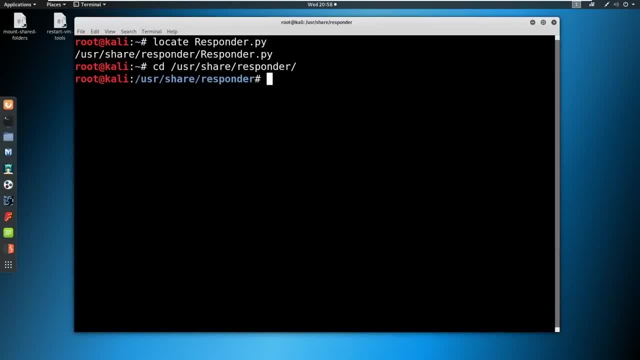 running as early as possible so you can get all the hashes that you possibly can when people are coming into work and logging in, generating traffic, making noise. Somebody asked what's the name of the attack that I just explained, So it is known as: 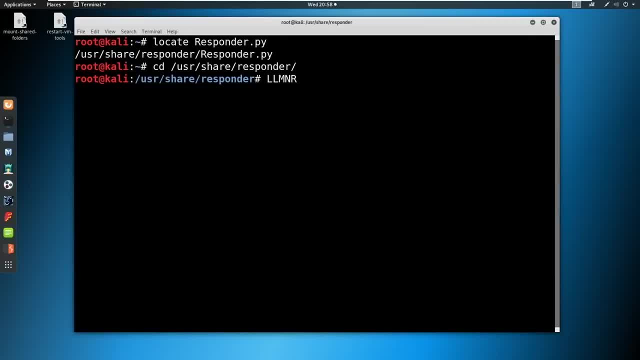 I'll type it out here: LLMNR or MBTNS poisoning Like that. Now, I can never remember the full command, so I'm going to cheat just a little bit. All right, So we're going to fire up responder here and we're going to treat this just like. 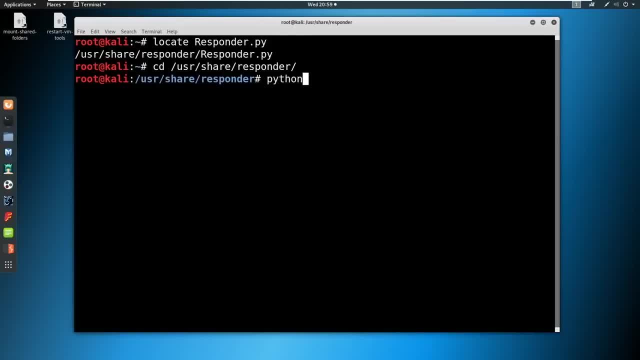 an internal penetration test. So we're going to say Python responderpy. You're going to do a dash I for your interface, Capitalize, If I can capitalize. You're going to say eth0 and then switches of R, D and W. 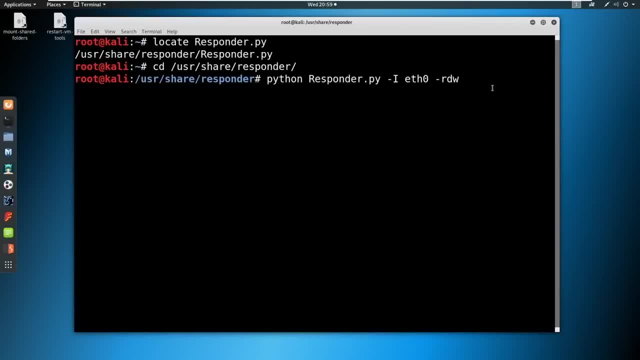 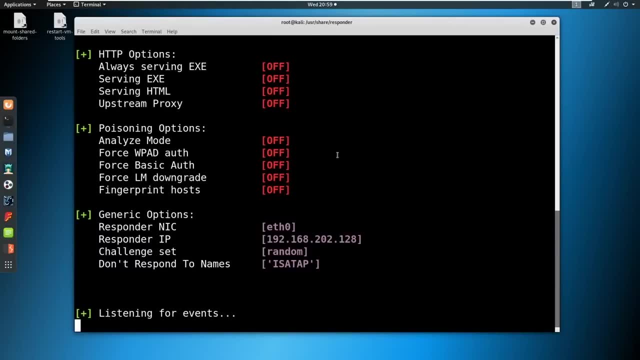 You wouldn't see this responder in the OSCP at all, because this isn't an internal technique. Typically, the OSCP is capture the flag slash external technique. This is focusing on active directory. Your settings should look very similar to this. So if you didn't catch this, 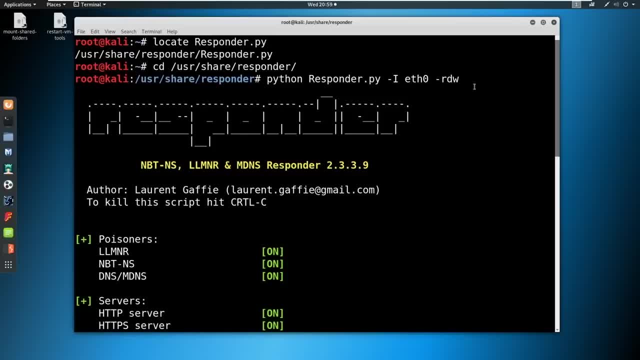 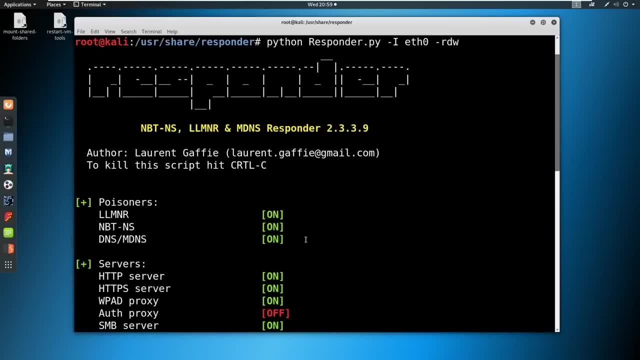 responderpy: dash I eth0 dash R D W And you come in here. you should have LLMNR, MBTNS and it's doing DNS poisoning as well And it's got all these different servers on, So we're not. 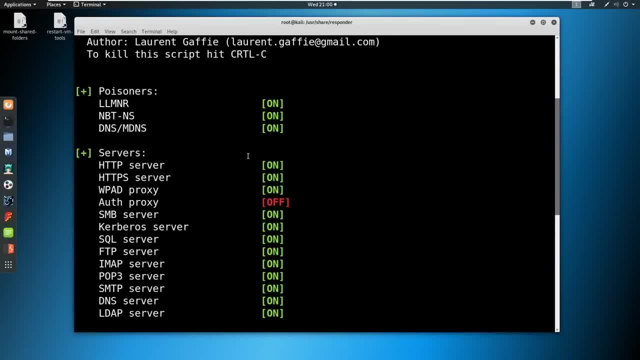 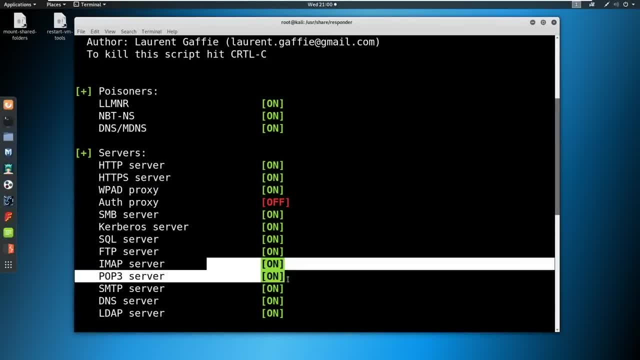 We're listening to the OSCP. We're listening to the OSCP. We're listening to the OSCP. We're listening on HTTP, HTTPS, WPAD, IMAP, POP3.. You name it. we're poisoning it, except the auth. 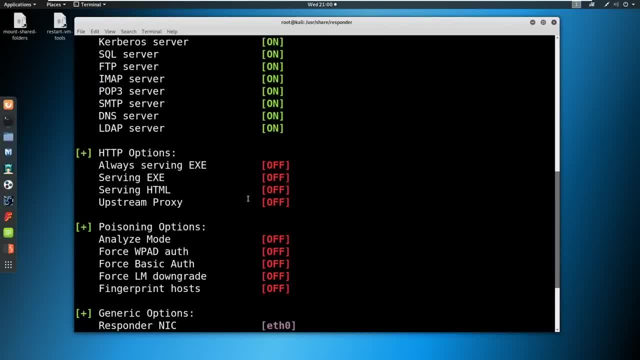 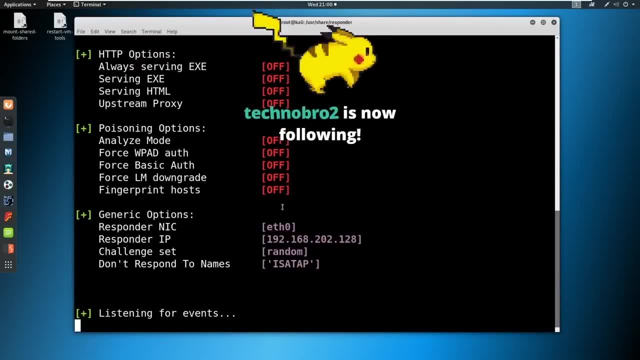 proxy by default? We're not, And then we have options if we want, but these are off by default. That's absolutely fine, All right. So we're listening for events. Now you might start to see some events come across in my household if I did things or something's starting to talk. There's. 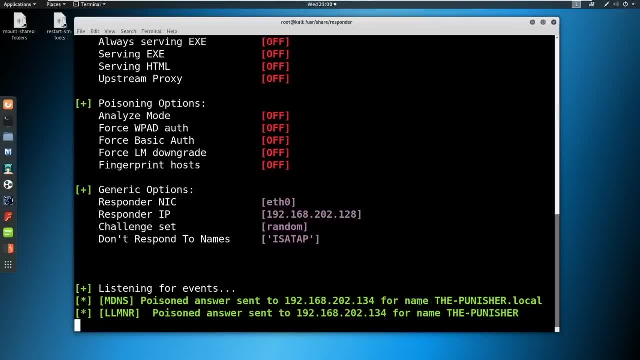 one right there. The Punisher just did something. The Punisher just sent out LMNR for something, or MDNS, So you just saw an event come through. Now that's not a hash, That's just an event. So you'll see a bunch of events and occasionally you'll get a hash. 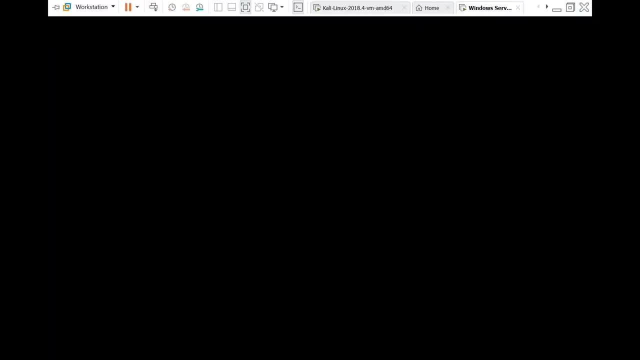 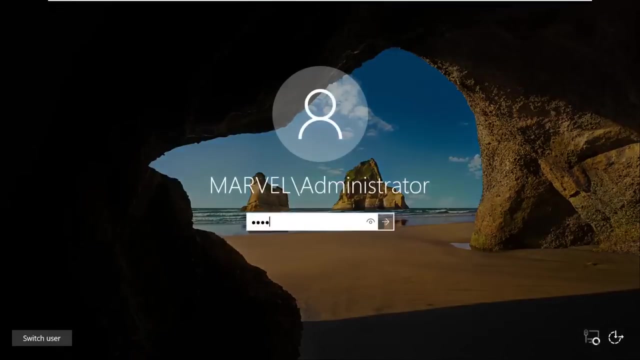 So let's look at if we can trigger another event here. Ah, it may have been actually locking itself. I have no idea what just caused that. My password's incorrect. That's not good. Oh, it's administrator, I'm locked out on the domain. 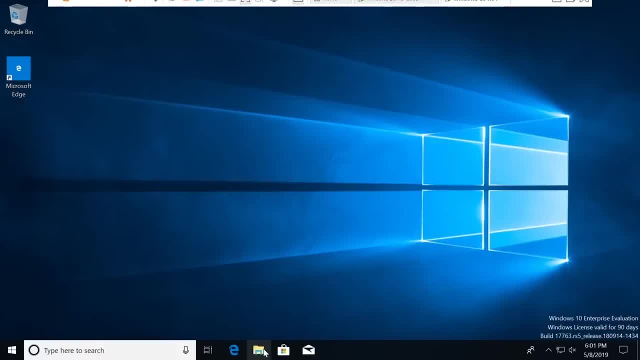 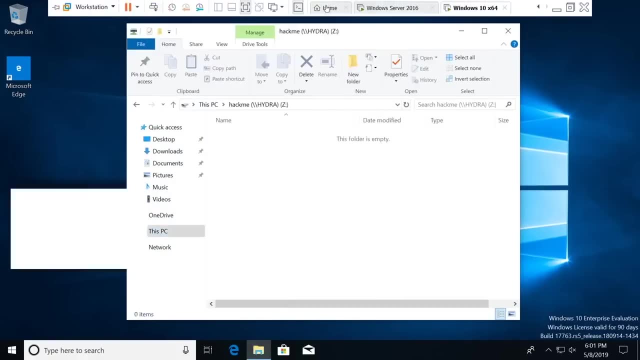 I want to be on. Sorry, I want to be on this guy. So if we come into here and we go into our PC and we just try to access this HackMe, let's see if that generated anything. Yeah, So we just. 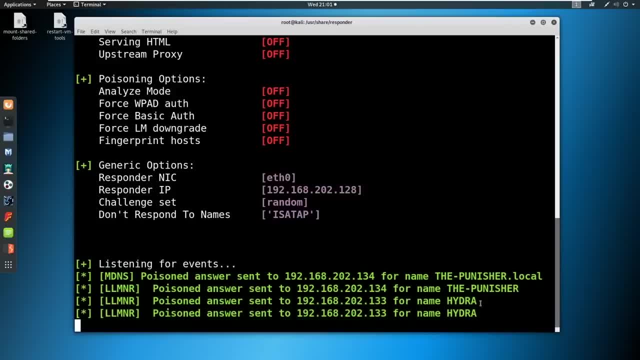 We just tried to connect to Hydra and you're going to see that we sent something to Hydra here. So you're seeing these events come through, And now what we're going to do is we're going to push this along for proof of concept. If you're sitting in a network, eventually you're going to get 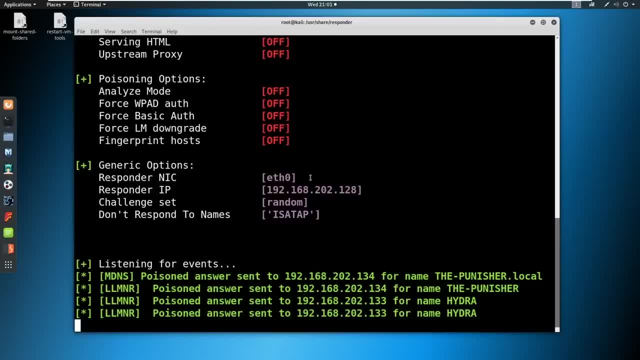 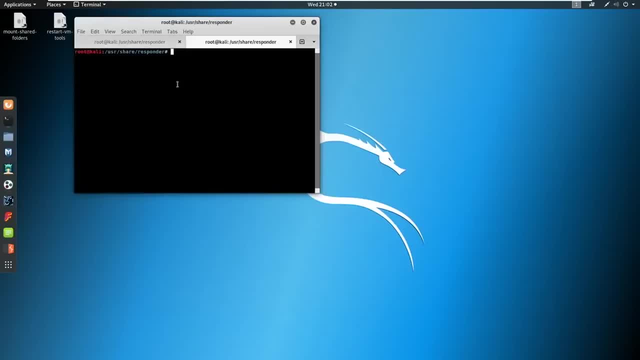 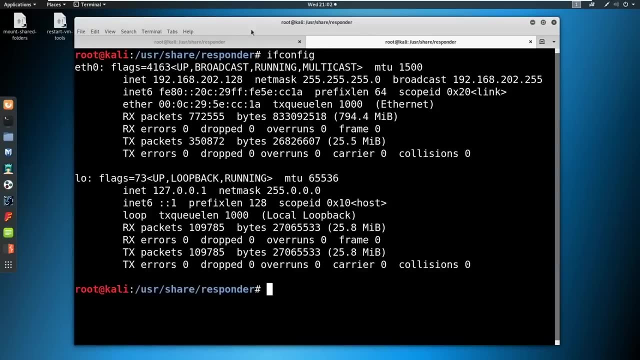 something coming your way. But because we're not sitting in a network, we're just going to, We're going to force it along just a little bit. So what I want you to do is go to File, New Tab, Make it really big for you guys, And just say ifconfig And copy your IP address. 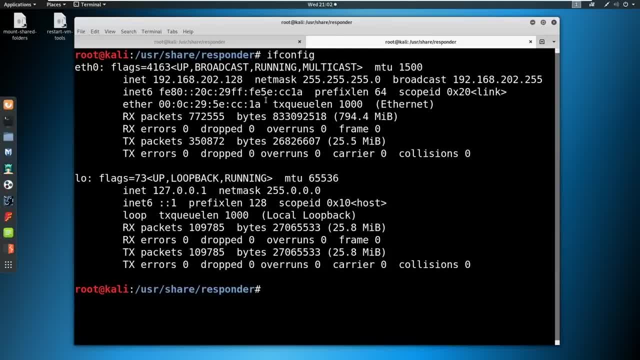 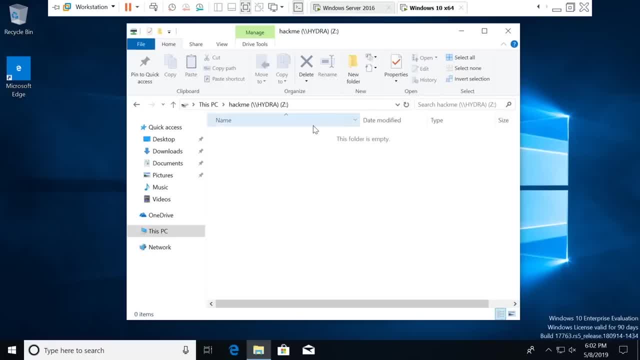 192.168.202.128.. Copy. I don't know if this is going to paste over, but I'm going to cross my fingers and say: let's do it All. right Up in the bar here we're going to just put the IP address. 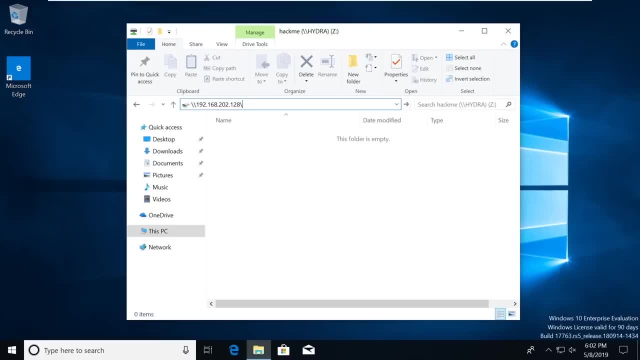 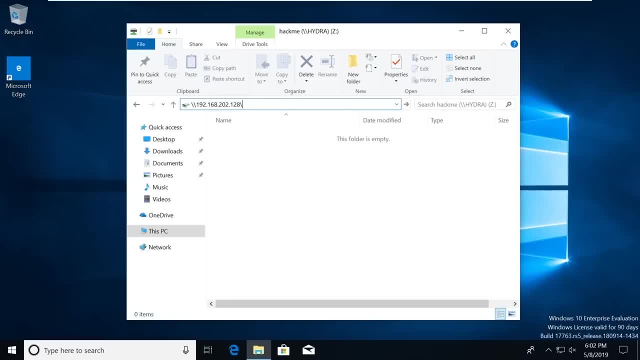 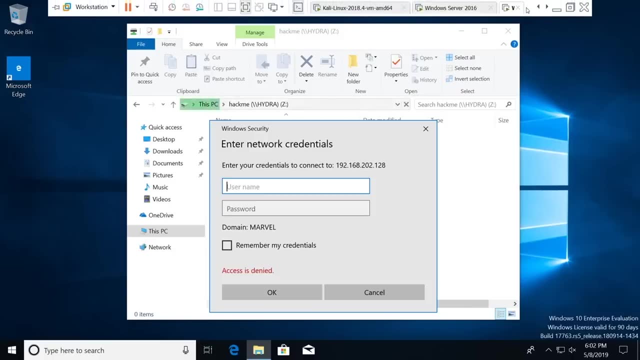 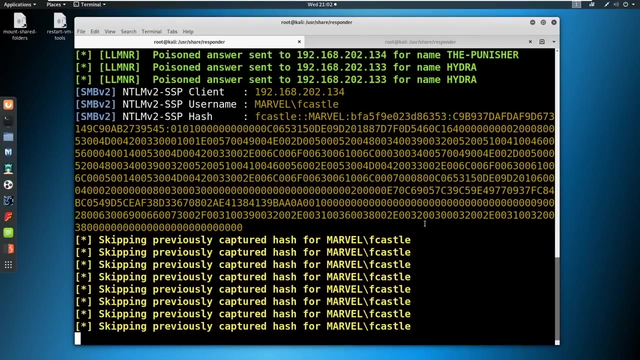 instead of our hacker machine And just hit enter. It's not going to be able to get into it, But if we go back, There we go. It just sent a shit ton of hashes. It skips them once it already got one. 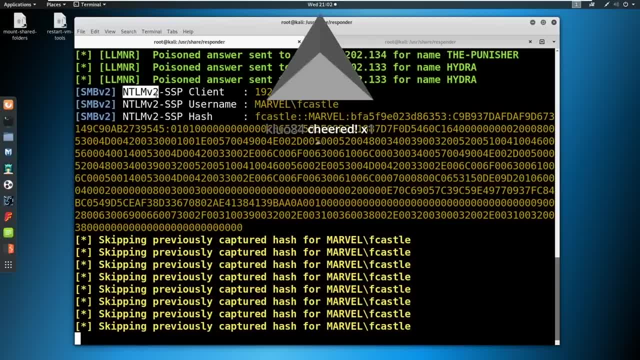 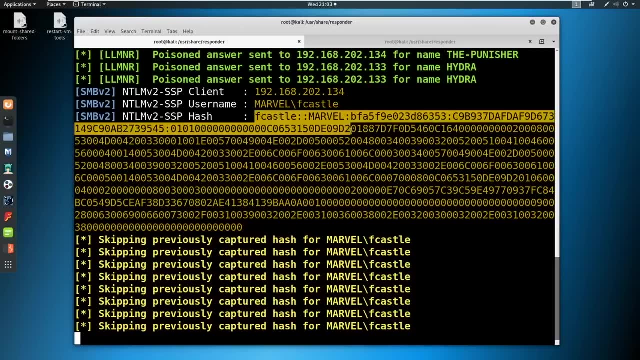 And you can see. now it says: hey, we got an NTLM version 2 hash, We've got The username of fcastle. And then you can see it's got the username, the domain, and then this is the hash. This is the NTLM v2 hash. Let's copy this bad boy, Shall we. 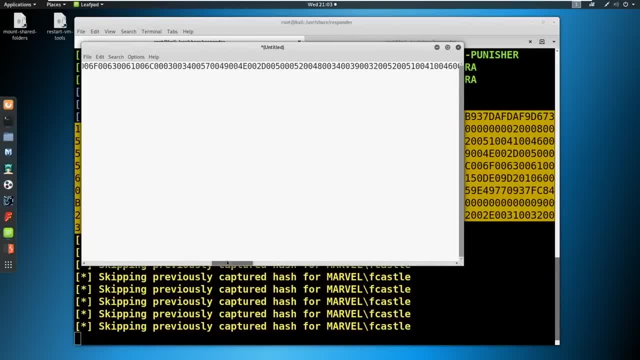 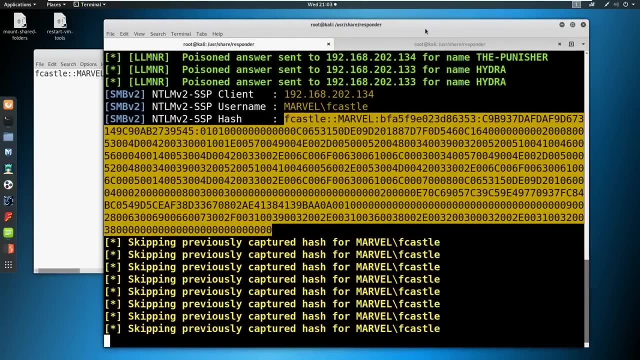 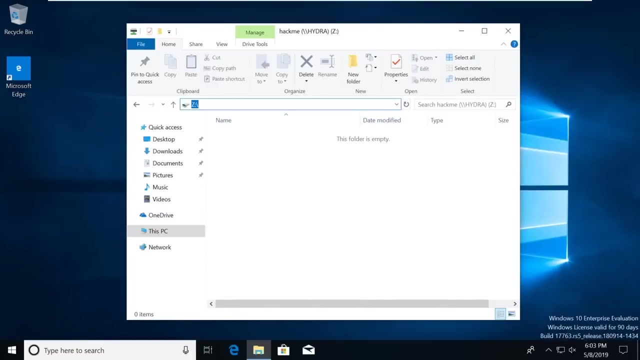 Just paste it into a file for now. Okay, Let's talk strategy. Hey, Gabe, Thank you for the sub. I appreciate that. Okay, So strategy here. Strategy time. You saw me point this maliciously at myself. Right, We went in there, We typed in the IP address. 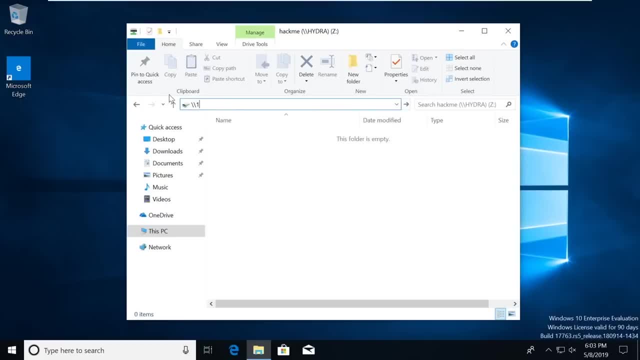 It's probably gone now. It is because it didn't resolve, So we can do this on a pen test. We can absolutely do this on a pen test. One place that I really love to use This is if you find default credentials, say like on a printer or anything that has. 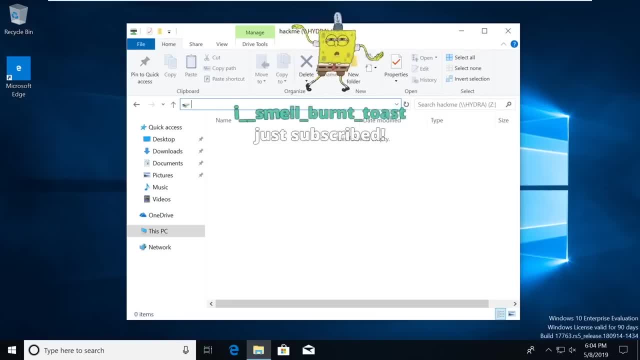 configuration abilities. Thank you, Burnt Toast. I appreciate that. So if we find this anywhere that has configuration abilities and it allows us to store credentials, sometimes you'll see like a printer. Let's give an example: A printer And it has an SMB share. 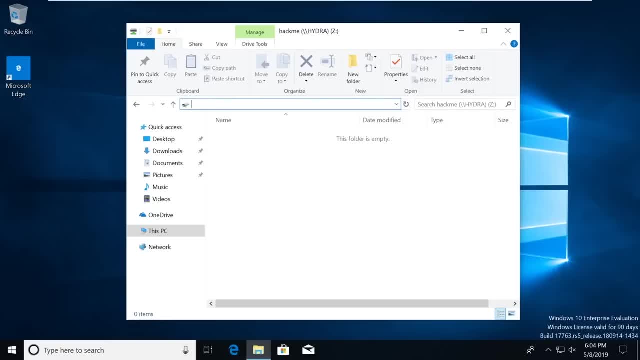 Now you can't see the username. You can't see the username and password for the SMB share. It's typically it's hidden, right, It's a bunch of asterisks or whatever, But sometimes it says, hey, what server? or what. 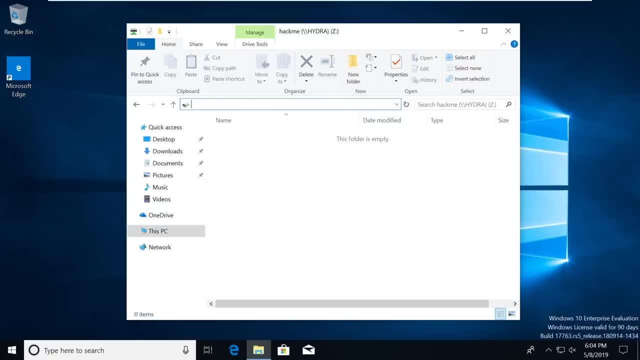 computer do you want to send this file to? And you say, okay, here's the IP address. And a lot of times it has this test button. If you've ever set it up, you can test the SMB share connection before, or you can just save it. even Both will work. 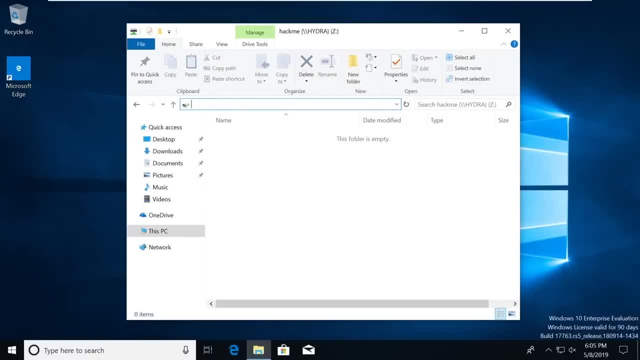 You put in the IP address of your computer instead of the computer it's set to, and guess what? The credentials for that SMB share user fly over to you. Now, a lot of times people aren't using least privilege and those SMB shares have. 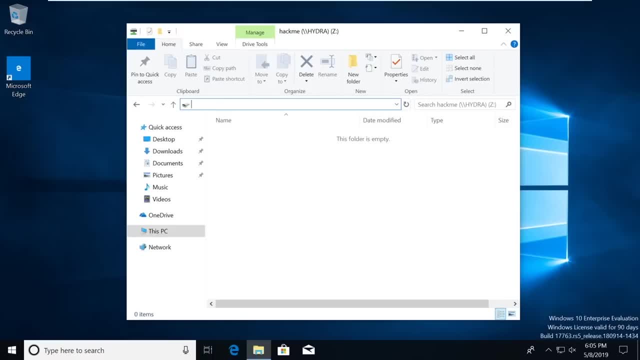 escalated privileges and are giving you instant win. The same thing happened not that long ago on another server. I don't remember what it was. It was some sort of VPN that I was able to log into- bad already with default credentials, But they had basically a domain account just sitting. 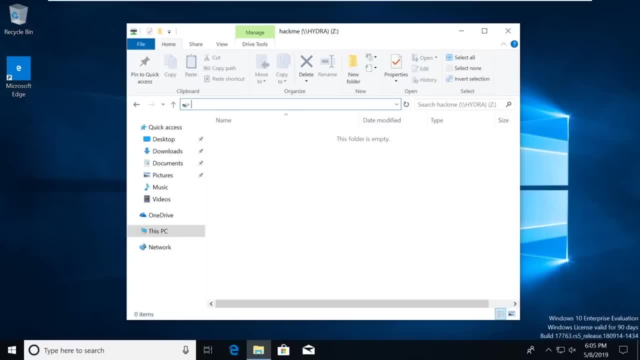 on their server And they had a domain account just sitting on their server And they had a server that I pointed to myself, was able to crack it, and the password was like Starbucks, something or another. So it went down really fast. It wasn't complex at all And we'll get. 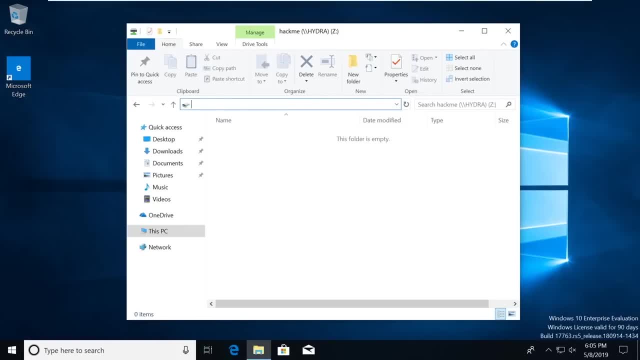 into defenses here in a second. But when you're running Responder and you're navigating around the network, if you're finding things like that, those are situations where you should say: aha, I can point this to myself and capture this hash. All right, now we have two options. We've got the 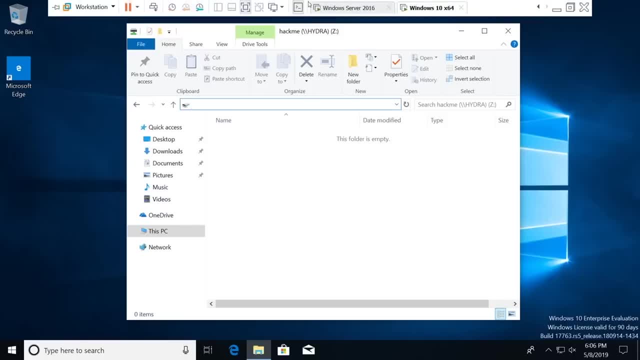 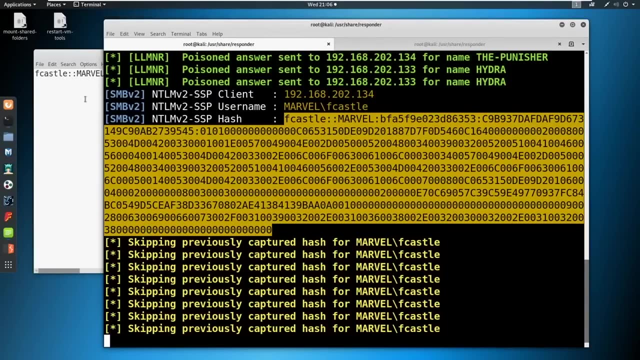 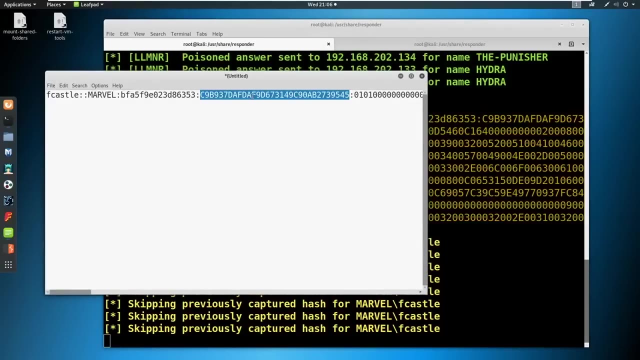 hash. Let's go back and try to crack it. So I'm going to save this file out. Actually, what I'll do is I'll copy this, And this isn't going to work. I'm going to show you how to potentially get it to work for your system. 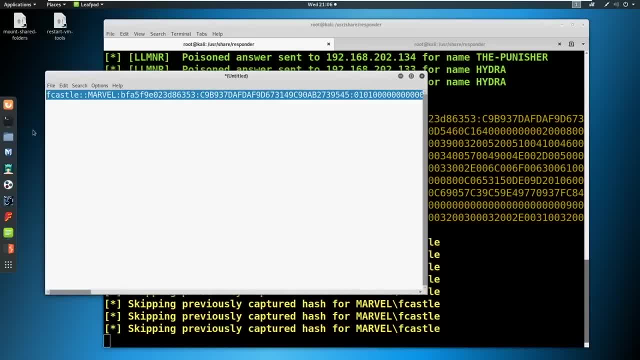 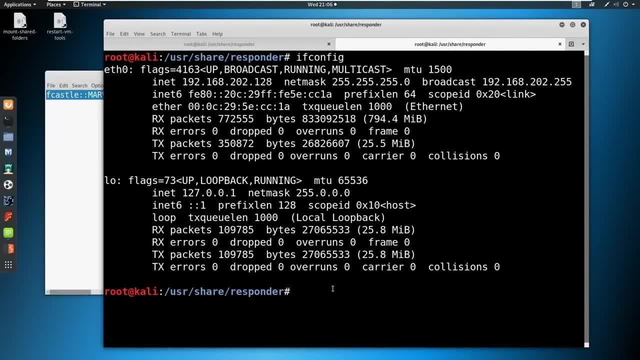 It could take a long time. So let's do this. I'm going to go back and try to capture this hash. come into here and let's just go and say we're going to say gedit, hashtxt. I'm going to paste. 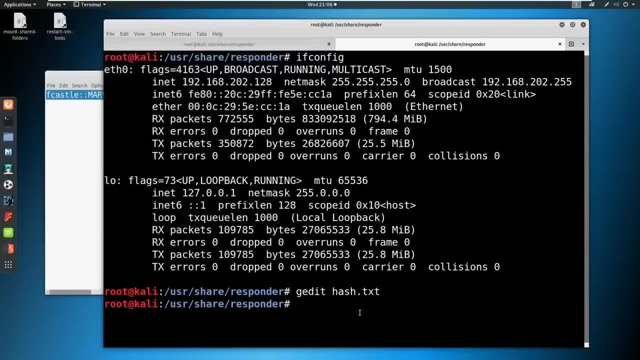 that in there and save it. Now, if you ls actually, let me locate rockutxt. All right, So something I've done on this computer that you may not have done already, and this is I'll talk for a minute so you guys can have time to do this. If you type in locate rockutxt, typically you 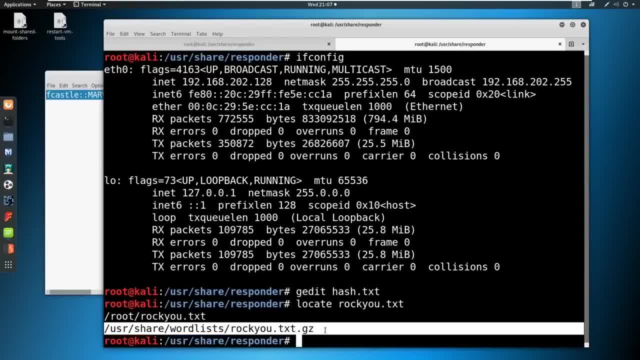 have a user share word list rockutxtgz. It's a zip file. Open your folder, navigate to that list, to the zip, and unzip it. It is a large, large password list If you've done any sort of basic. 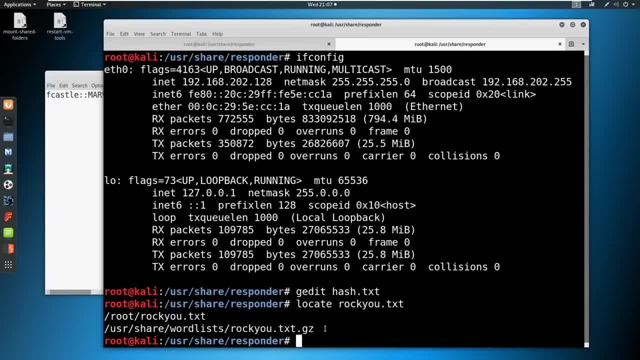 hacking. you've probably seen this. If you haven't, it comes built into Kali by default. It's not the one that I run. I use one of the larger sec lists. I'll have to dig it up, but it's like in the billions as opposed to. I think this is maybe in the millions. 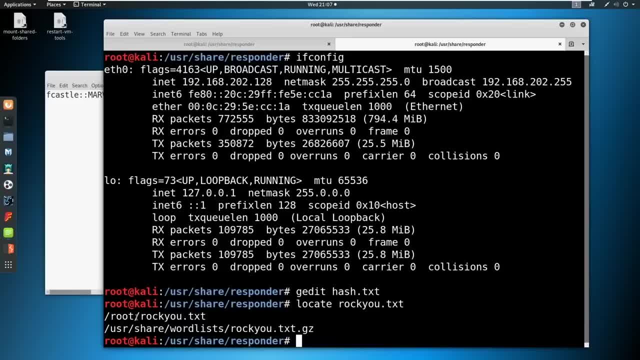 of word lists. So go ahead and just get that unzipped, and then I've got mine sitting in the rockutxt here. but I'm going to use hashcat on my machine, I'm pretty sure, unless something's changed. 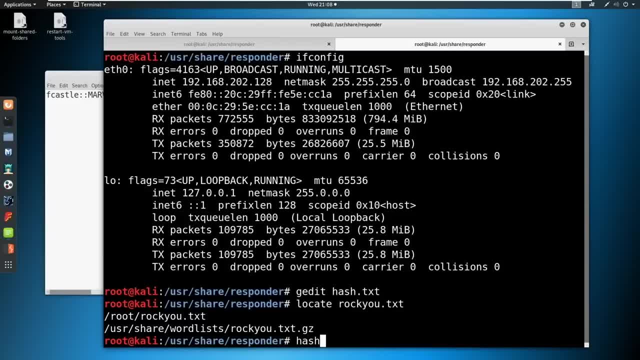 So what we're going to do, though, is we're going to say hashcat, and then we should just say: m Actually, let's do a dash dash. help so I can show you what we're doing. So you need a dash m? It's basically a code, right, And these are all your m's, if you. 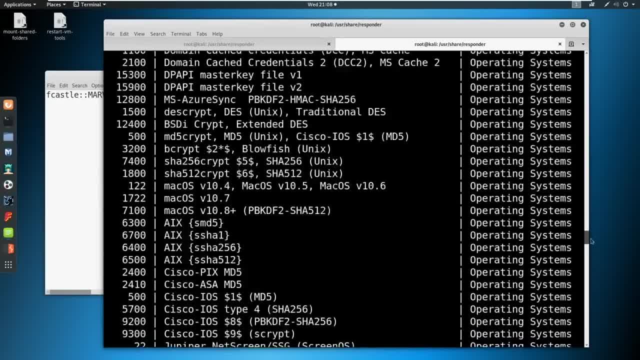 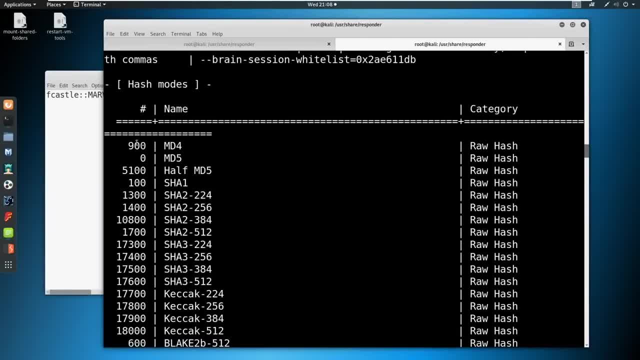 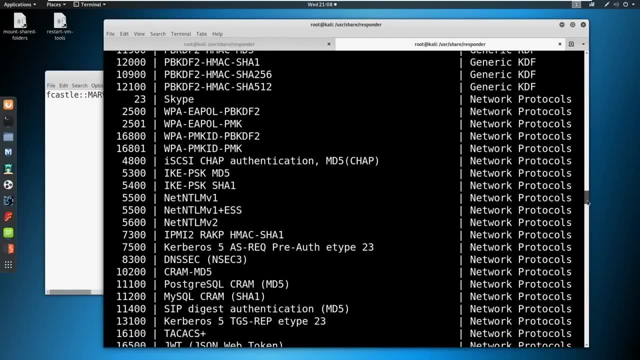 come into here. Yeah, these are still all m's. So all of these are the different type of hashes, These are modes. I guess the m stands for mode- All different kinds of hashes. If you come down into network protocols, ntlmv2 is here. It's under the mode of 5600.. So 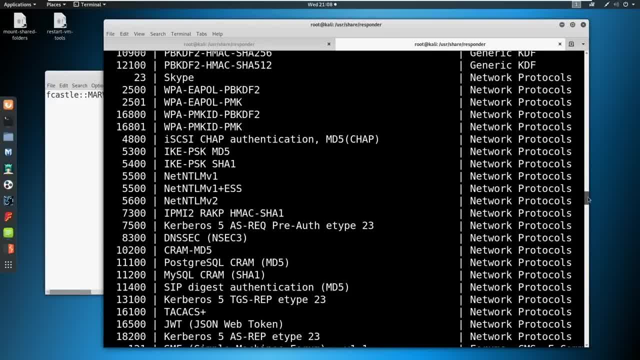 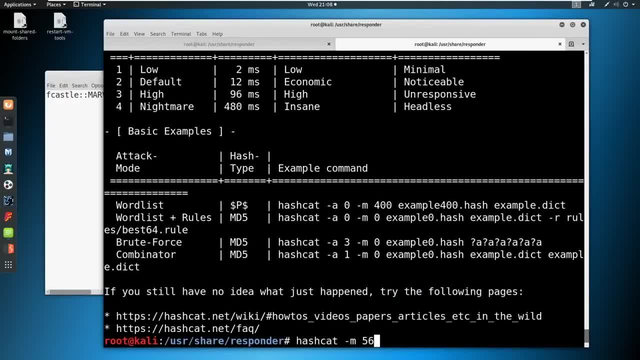 we're going to be using 5600 for this one. So if we say hashcat, dash m 5600, and then typically it wants your hash and then it wants a, a password list, we can say root, and then we could say rocku dot text and hit enter. 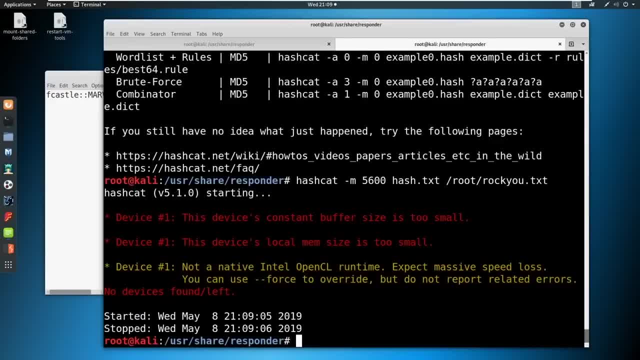 We're going to run into an issue. First issue is: if you're running on a VM, you're not going to be able to run this without using a dash dash force. So if you're following along on a machine itself with Kali installed directly, good for you. 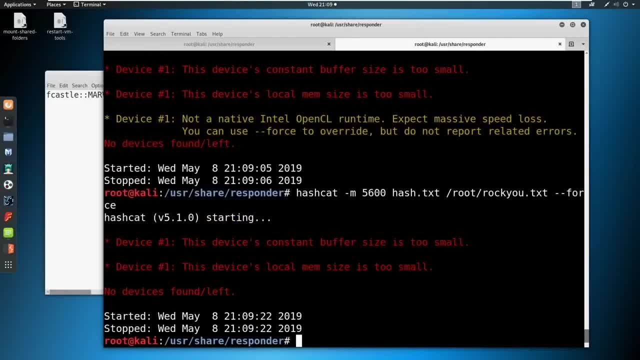 You win the internet, So you could try dash dash force. Mine will not work. I am on a 9000 series i7. and it worked on a 7000 series. It does not work on this anymore, So if you're on a newer version, 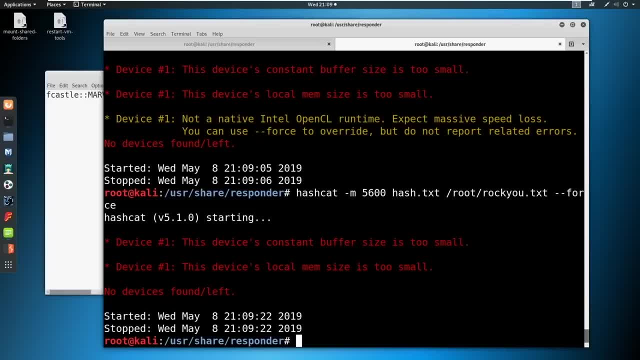 of a CPU, you may run into this issue. So the alternative anyway, and let's talk about this strategy too. I'm on a gaming computer. I've got a 1080 Ti. If you try to run this on a VM with, 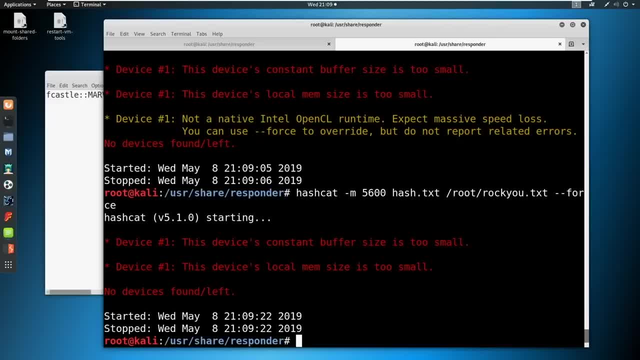 the dash dash force. it's going to take a while to go through rockytxt. If you are doing labs or anything, any type of type of pass or cracking, and you have anything of a decent, it doesn't have to be anything expensive- a decent graphics card, it's going to go through this rocky list. 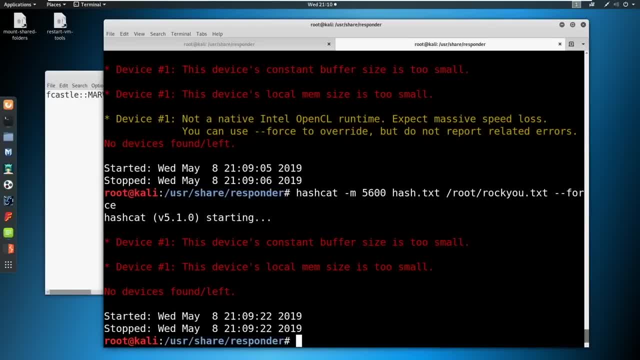 really fast. So something to think about. when I was doing the OSCP labs, it was taking me hours to run through rocky. I had a 970 at the time And it would take literally seconds to run through rocky. So something to think about there. So I'm going to do is I'm going to copy this hash. 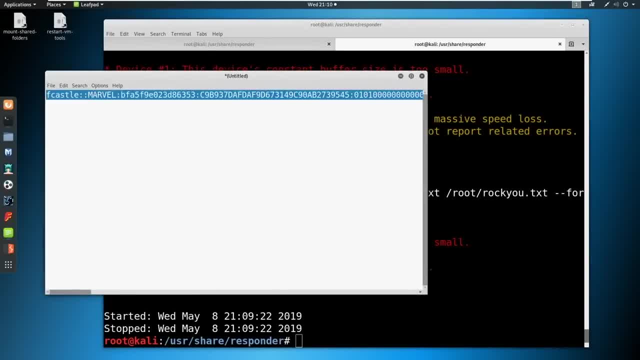 over here And I'm going to copy this hash over here And I'm going to copy this hash over here And I'm just going to put it in that same hash file. Give me one second here And I'll I'll bring. 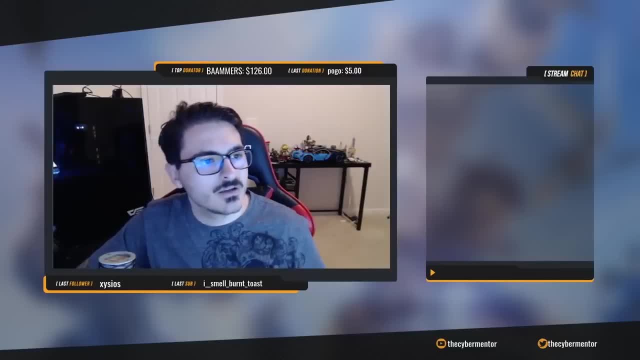 up my face. You guys have something to look at. I know you guys like it. Get to my hash cap folder. Paste that almost done. Can I share the sec list? Yeah, I'll share it at some point, You saucy minks. Thank you. Wow, So I'm running hash cap 4.2.1.. For Windows you can run whatever you like. I know at one point they were saying hash cat three was like the best if you wanted to run it on Windows. but I haven't had any issues with this. 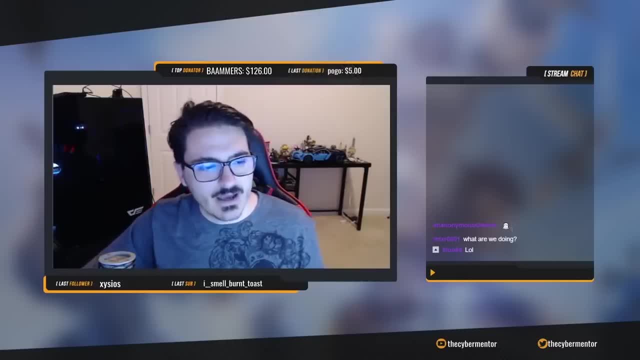 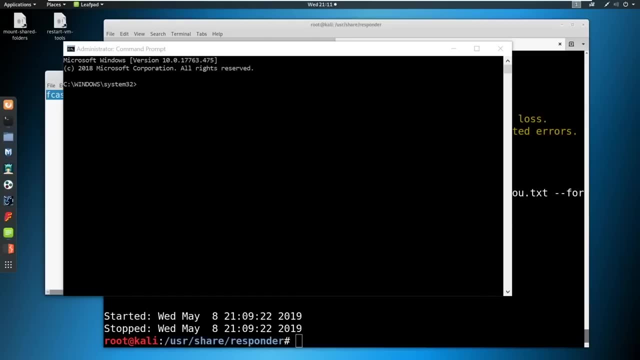 So go into command. I'm going to run command as admin And then I'm going to come back to the screen. All right, So cd users, he desktop hash cat. All right, Hash cat 64.exe is what we're going. 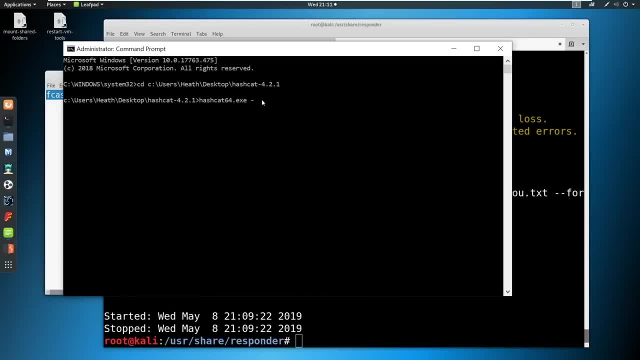 to be running Same thing, Dash m 5600.. If you don't get hash cat running, you can also use john. john the ripper will work on NTLM v2 hashes as well. So m 5600.. Got a hashestxt in here somewhere and then rock youtxt. 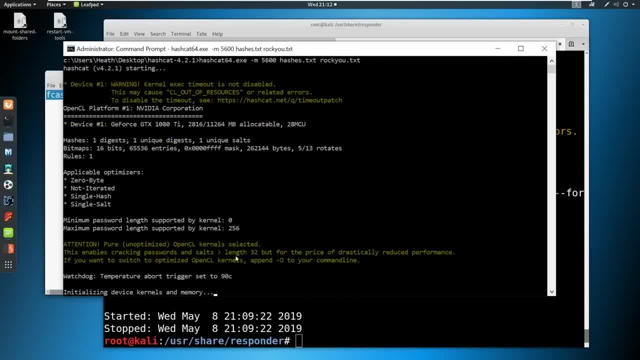 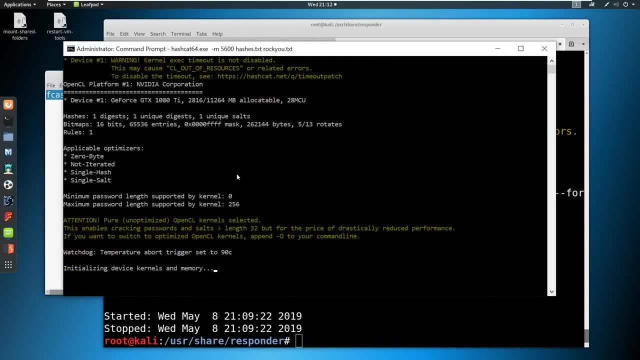 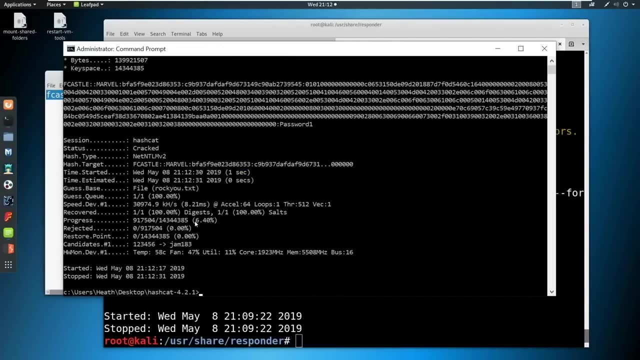 Okay, so it's going to start firing this off. It's going to take a second to load up the device kernels in memory and then it's going to fire through this and try to attack this hash. And that was it. It went through 6.4% of the list. 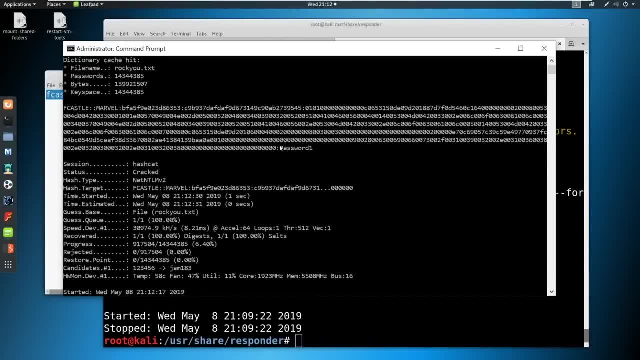 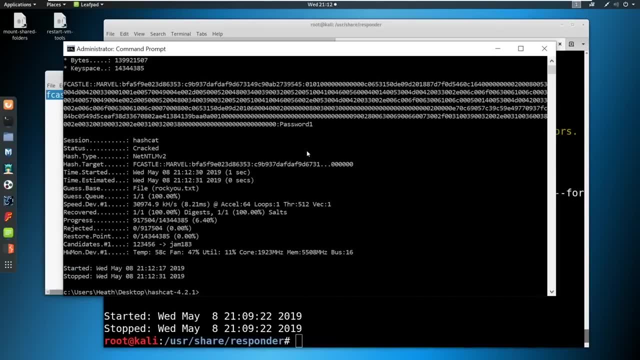 that fast And it also cracked the password, which was password one. So now we've got the password for the user Frank Castle And we're going to try to use that at some point as an attacker to navigate around the network. Now I'm going to leave it here for now. 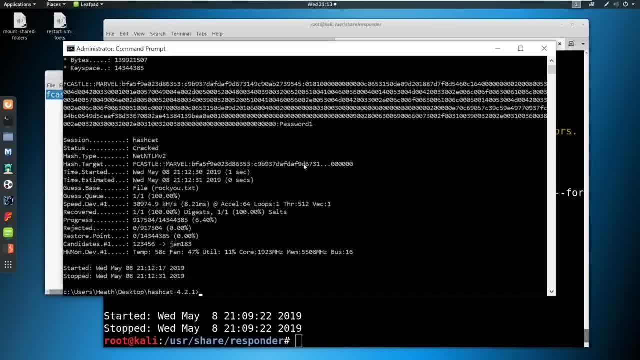 I'm going to leave it here Only because I don't want to go further. We're going to talk about all kinds of strategies. Next week's really going to focus on on hacking ad. Somebody asked about thoughts on AWS for cracking your other hosting services. They have hosting. 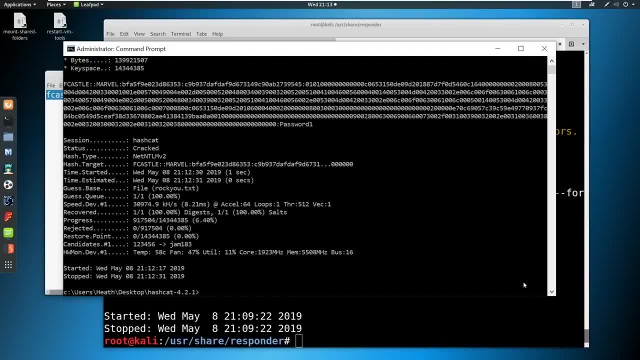 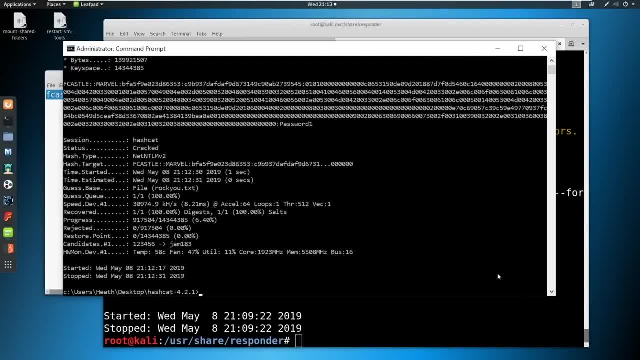 you're more than more than welcome to do that kind of strategy. I just have one locally that I like to use. Let me share my word list. Hold on, let me just get that open. You guys can look for it And that way I don't have to Google it and find it and everything else. Give me one second. 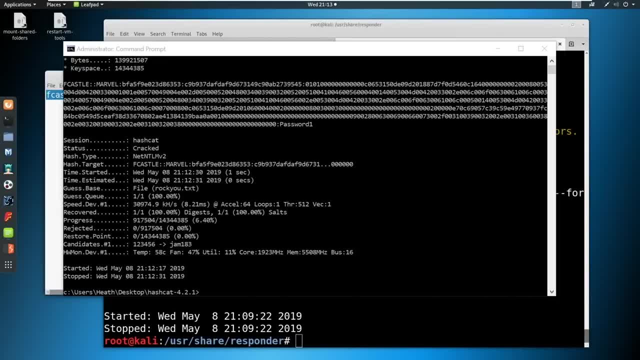 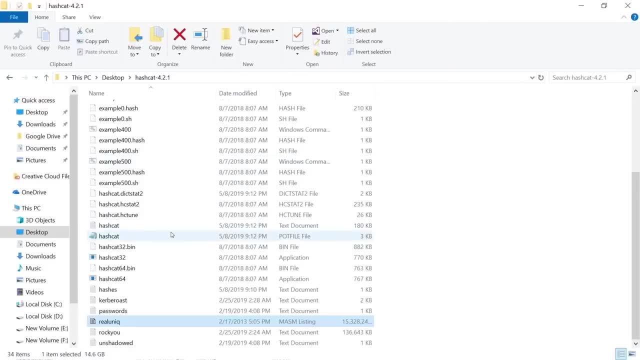 All right, the word list I use. Bring this over. It's called real unique U-N-I-Q, Real U-N-I-Q. That's it. It's a 15 gigabyte word list And it cracks quite a bit of passwords- Not the most effective. We've got some custom lists that. 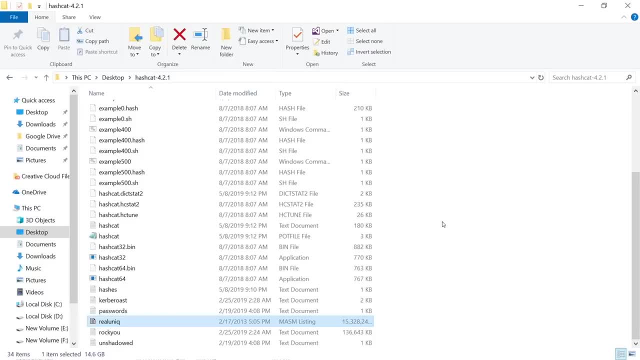 we use internally that I can't share with you guys. Uh, with custom rule sets and everything, And those work even better. But if you're looking for like a basic, basic list, this is a good one to start with. All right, let's talk one more thing. Let's talk about defense strategies. 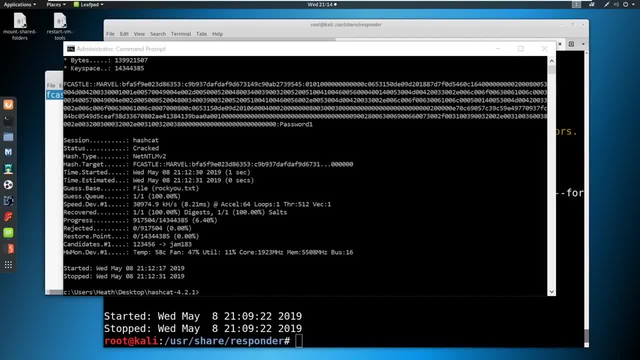 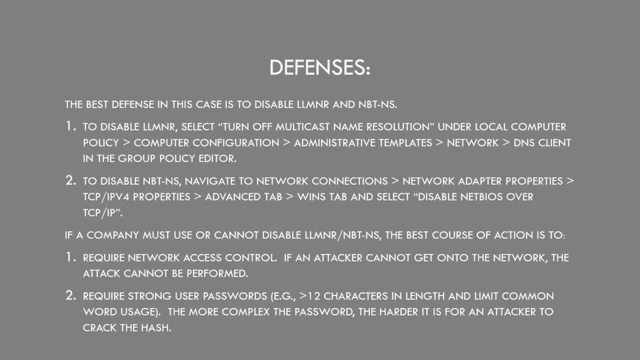 Let me bring up the PowerPoint so I can talk this through with you real quick. All right, so defenses. if you want to prevent this, you can disable LLMNR poisoning. A lot of admins do not like to do this, So there are other options as well. But if you want to know, how to disable LLMNR poisoning, you can do that here. So if you want to know how to disable LLMNR, you can do that here. So if you want to know how to disable LLMNR poisoning, you can do that here. 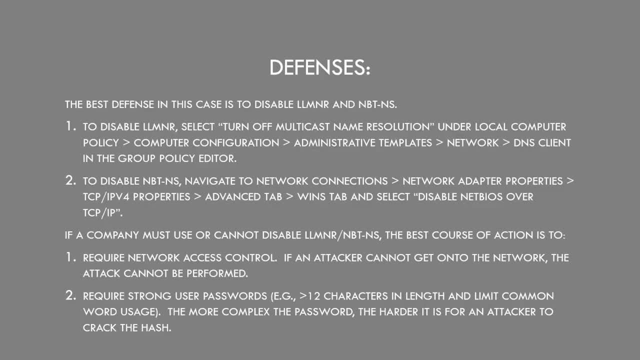 Here are the defenses for that. Also, you'll have to disable MBTNS, So we will navigate to those files in their proper locations and turn off, disable net BIOS over TCP IP and disable the DNS client in the group policy editor. So if you don't want to do that, 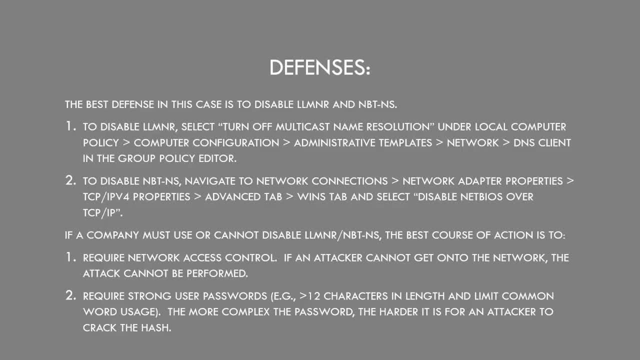 and you are thinking of other defenses. then what are our options here? Well, we can require NAC, We can do network access control. So if you can't get onto the network, this attack can't be performed. right, There's obviously there are bypasses to NAC, So it's not the latest. and 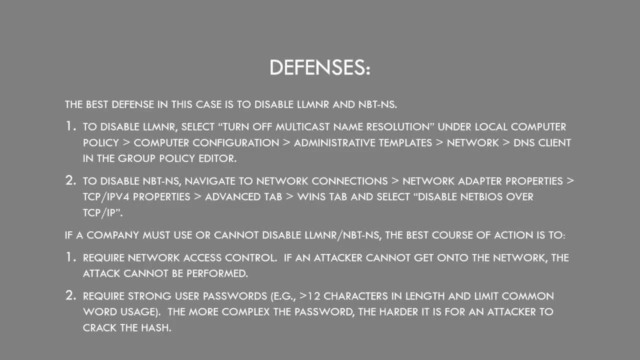 greatest, but it's one form of prevention. The other thought is to require strong passwords- Greater than 12 characters in strength- or in length is what is said here- and limit comment word usage. Uh, honestly, the longer the password, the better. If you've got a four, 40 character. 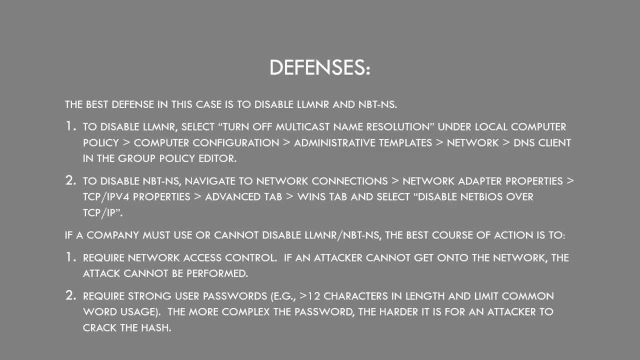 password, even if it's just a sentence. uh, we're not going to, uh, we're not going to be able to crack that. really, It's hard to crack anything over 12.. We have cracked 14 and 15.. 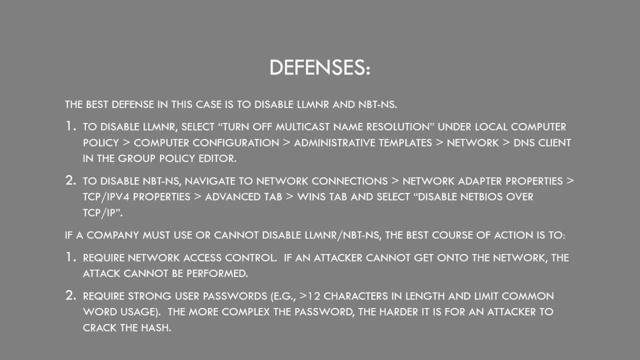 If you're using some kind of common word usage. uh, one that came up recently was a Bible verse, So don't think it looked creative Like it was a Bible verse, had a space in the password. I was impressed, but it still fell down. Um, these very, very common words like that, They'll fall. 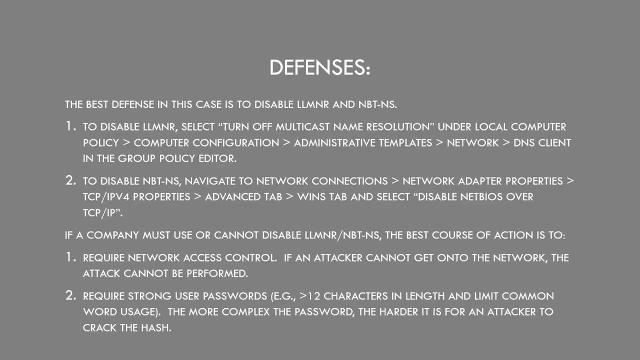 So the longer the better. I think mine's 20 something characters, uh, my coworkers in the forties, So just uh, just think of those strategies for defenses. So, with that being said, we are going to hit the break button on this. We are going to be done for tonight. Maybe we can. 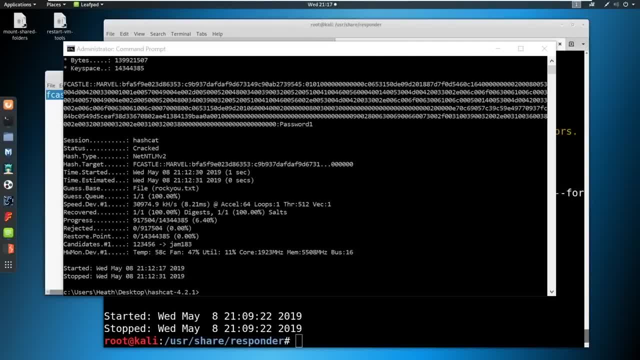 even get out early. Uh, next week we are going to uh focus more on the attacks and what we can do. We may even build our lab a little more. I don't have the lesson plan completely finished. Uh, we need to. 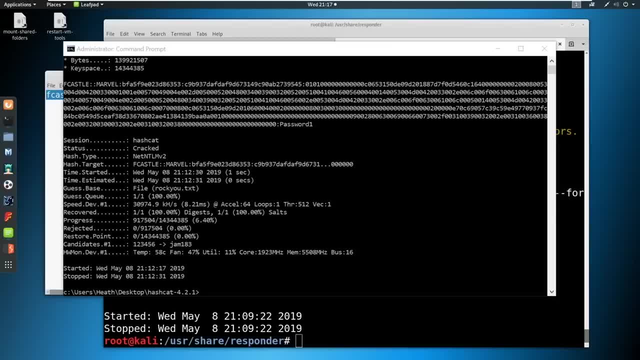 scan the network as well. That's something we haven't done. We haven't run NMAP, but I'd rather wait till next week to actually get a feel for what's out there, And then we'll just continue to build upon it. There's also some some things that I don't have set up. that, um, I don't know. 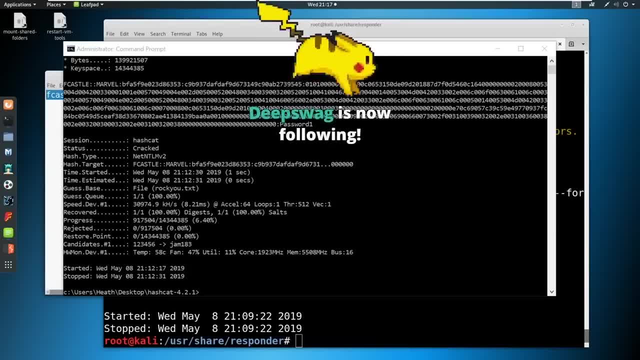 if I'm going to be able to set up. So uh, like, for example, MS 1710 or eternal blue. I don't know if I'm going to be able to like set that up, but that's something that you really commonly see in. it doesn't necessarily pertain. 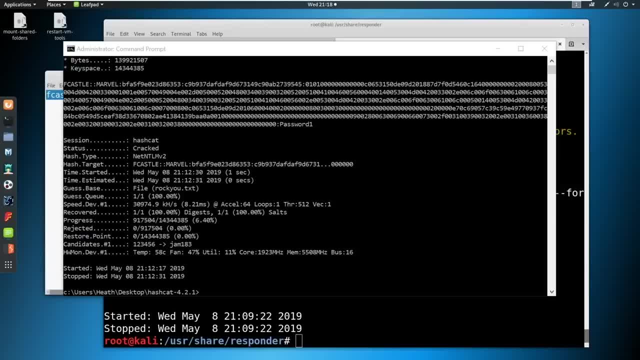 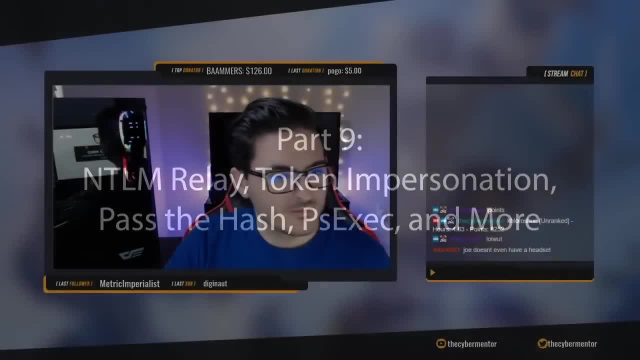 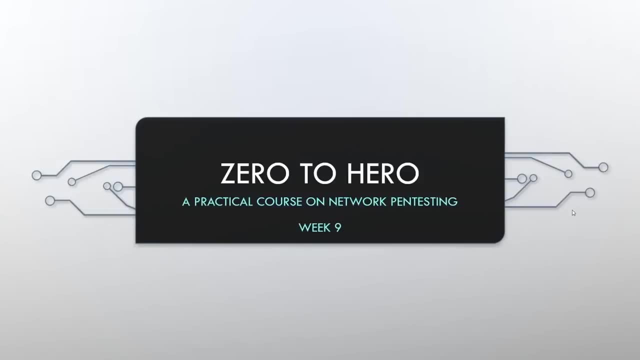 to active directory environments, but definitely pertains to things you would see in an internal environment all the time. All right, Welcome to zero, to hero. week nine. You guys are going to be able to make it through nine weeks. This may be the pen ultimate week. I have not decided. 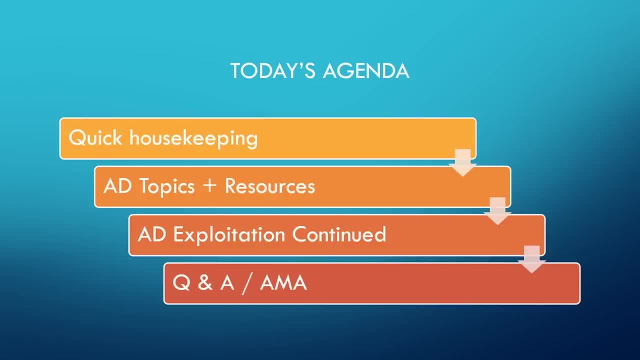 Hey, Nate dogs here. I haven't seen Nate dog in forever. What's up, Nate dog? All right, So today's agenda, quick housekeeping, and then we're going to go into 80 topics and resources And then finally we'll dive into our lab. do some 80 exploitation? continue that on. 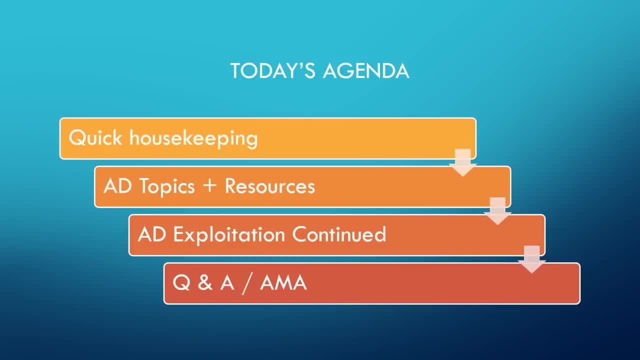 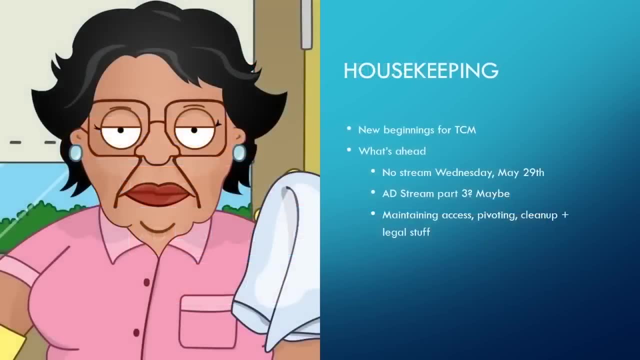 And uh, end with Q and a and AMA. I just thought you got arrested, Nate. That's all. That's all All right, bud. So housekeeping, first thing on the agenda. new beginnings for the cyber mentor. Uh, many of you have already heard some of you already talking about it. 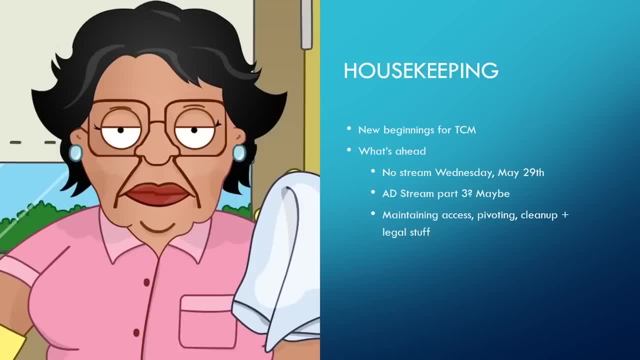 I put in my notice this week at my job and I am going to be starting my own venture. So, uh, don't know what that's going to be. I'm going to be starting my own venture. Don't have everything planned out, but I'm trucking it on my own and, uh, and you know, 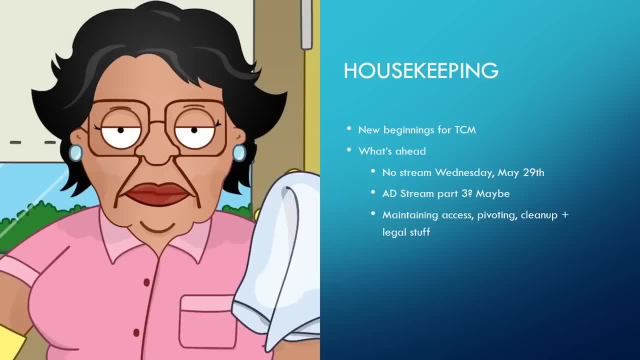 going to give it a try, So wish me luck And in this venture ahead. I'm sure you'll be seeing posts about it uh coming in the near future And uh I also plan on on blogging about the experience. So hopefully you guys uh may learn from my struggles on what it's like to uh run. 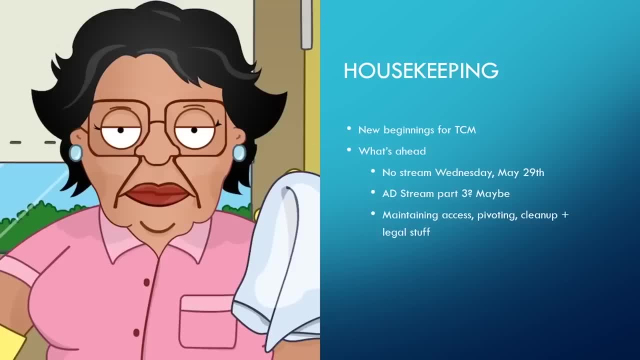 and operate a small one person business. So, uh, I'm going to be starting my own venture. So, other than that, let's talk about what's ahead. No stream- Wednesday, May 29th. Again, no stream- Wednesday, May 29th. I said this last week, I'll say it next week because somebody will. 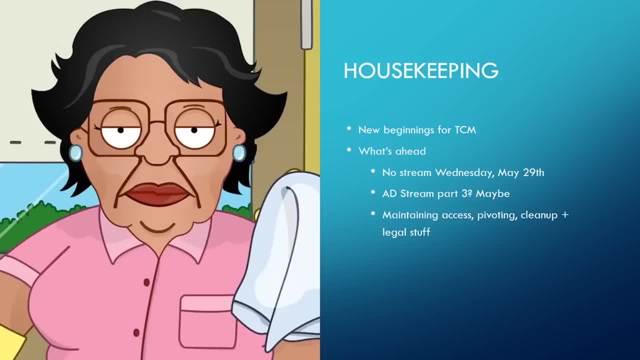 forget and show up. I will be out of town. I will not be here on the 29th. Now we have the opportunity for two different paths. We can either be doing an active directory, part three, next week, or we can go. 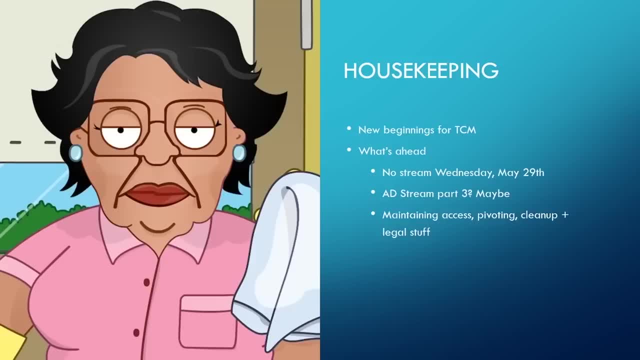 we can go right into maintaining access, pivoting cleanup, plus the legal stuff. So I'm going to leave it up to you guys And I'm going to. I won't know until next Monday what we're going to be doing. fully, I'll plan for both. Um, we're at a situation where 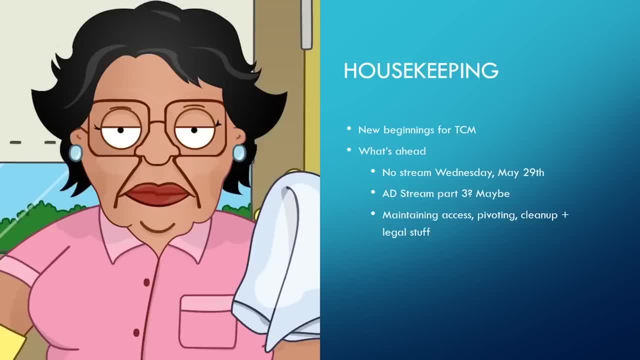 I have more than I could teach you. I could teach you weeks and weeks of active directory exploitation, Um, the issue is I don't have a lot of time to to build out the labs, So there are a couple of hack the box um machines that I'm going to ask you to upvote. 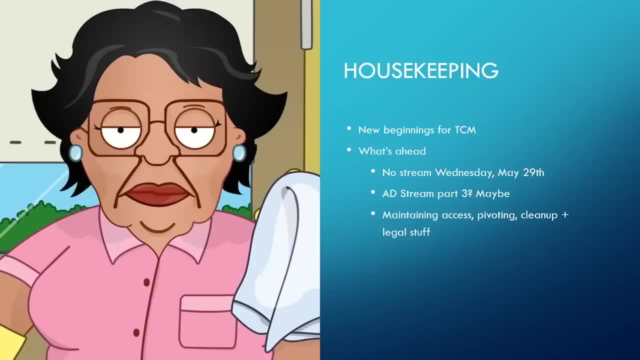 If you have VIP, I've already sent that out in the email. Uh, we'll talk about that here in a minute. If you upvote those, we'll have a third stream on AD and we're going to talk about um. 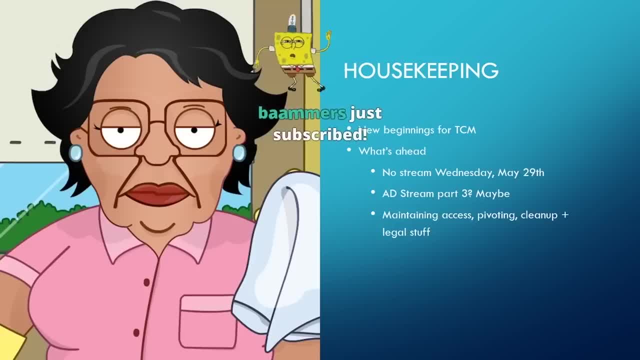 Kerber roasting and we'll talk about GPP and C passwords. We'll talk about eternal blue MS 1710.. So, uh, we have a lot to cover in another stream If we want to go that route. uh, still may be the last week. I don't know how much I have to cover in a maintaining access. 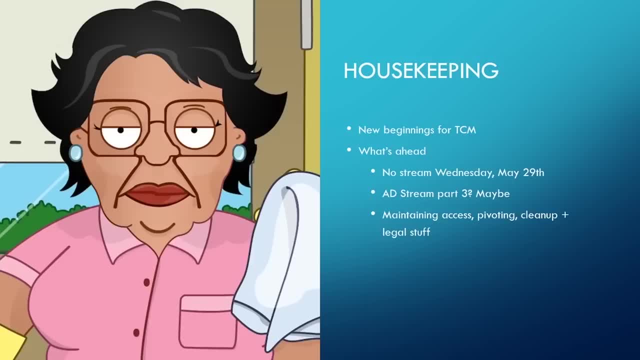 pivoting cleanup side of things. Um, plus the legal stuff, We may just do a super long stream, or we may do a special stream on like Tuesday May 28th and just have some fun with a- uh, with a legal document. We'll do something with it, Maybe play a drinking game out of it, or 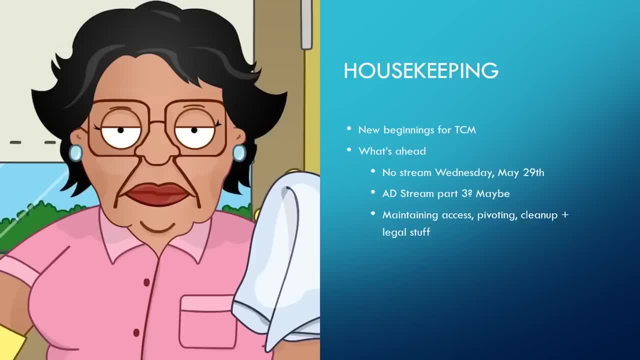 something and get, get me drunk before I go on vacation. So, uh, we'll figure a way out to end the course. So, uh, I'll see you guys next week. Bye With a, with a bang, and, uh, congratulations to all of you that have have made it this far. So. 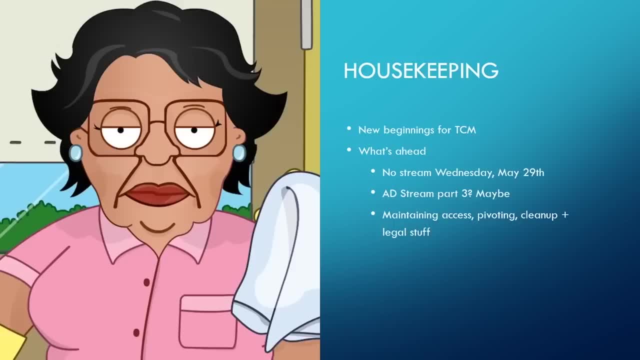 big, big hats off to you who've been here every week. Uh, I don't know if you realize, but we started with probably- I don't know- a hundred viewers on average- and uh, it's sexy in the beginning- and consistently, 50 of you have been here in and out every week. I think the 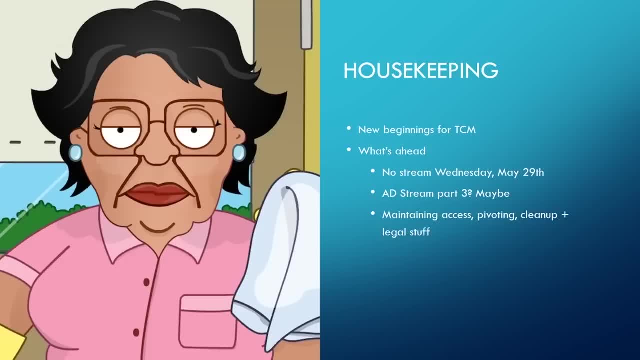 mailing list is somewhere around 500.. Um, so I know some people can't make it, but the, the ones who did show up in the beginning, they're going to be the ones who are going to be the ones who, in the first few weeks, you know they didn't stick it out, They didn't have that mentality. 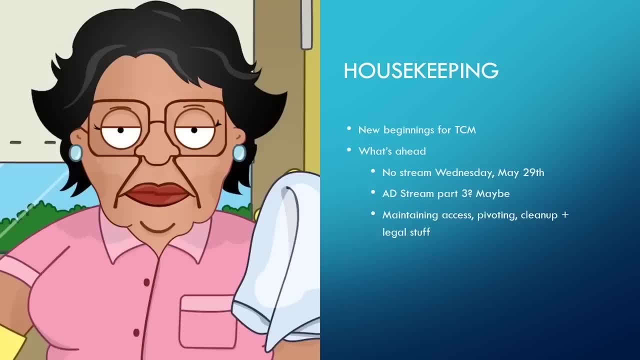 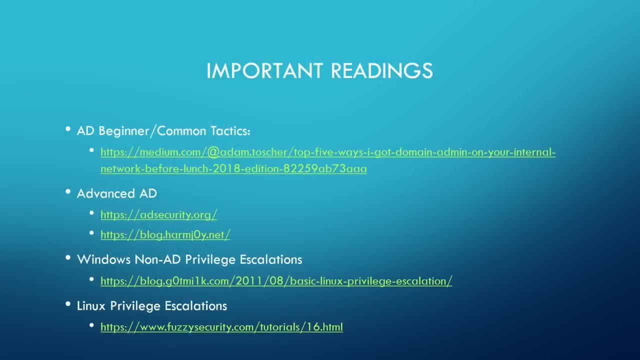 to continue, And you guys have continued. So big hats off to you as well for for sticking it out. All right, So let's go ahead and move on. First things first. I am going to give you guys some important readings, So I've already sent. 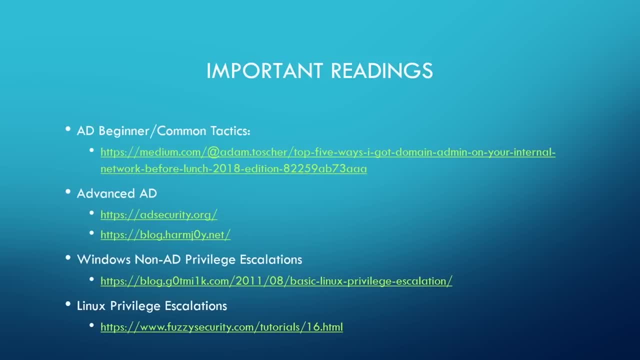 out some of this, but these are very, very important. Uh, the first one here is this: AD beginner: common tactics. It's the top five ways I got domain admin on your internal network before lunch. It's from 2018.. It still holds true. uh, fairly well. 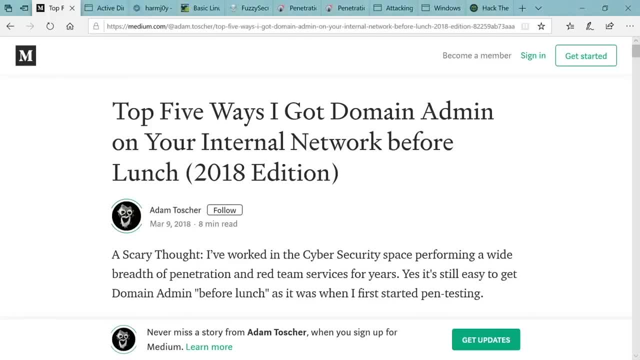 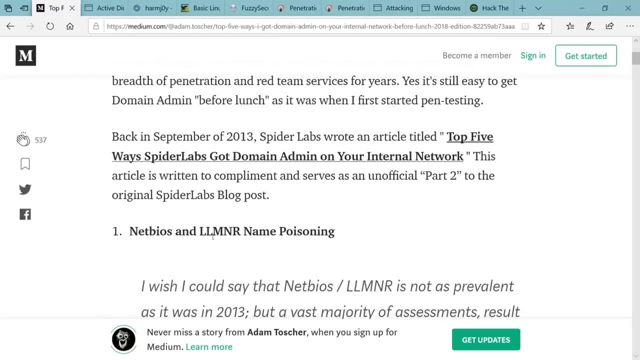 for internal pen testing assessments. Let me pull this up here. This is the article. It's really good. So if you scroll through it, number one: net bios and LLM and R poisoning. what did we do last week? That's exactly what we did. This is the number one method. It will hold true as number one. 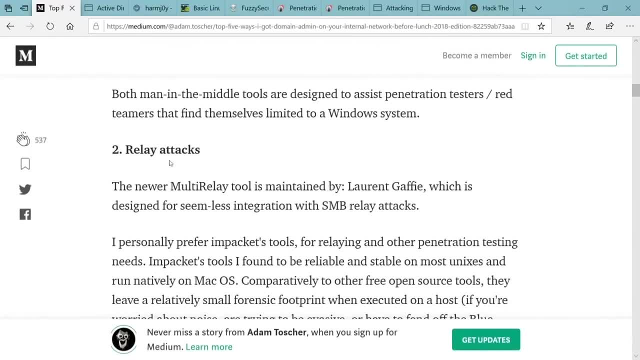 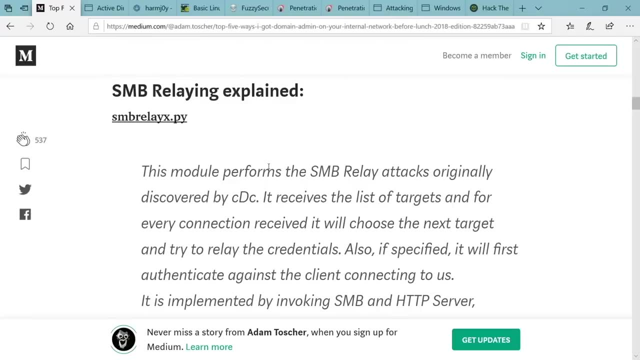 For quite some time scrolling through it. relay attacks are going to be covering relay attacks today. That's why I asked you to download or install a fourth machine. I know that's very Ram intensive. If you do not have the Ram, you'll just have to watch. Uh, so I have a fourth machine. 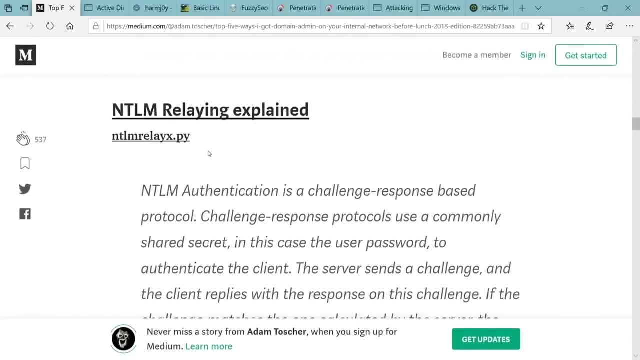 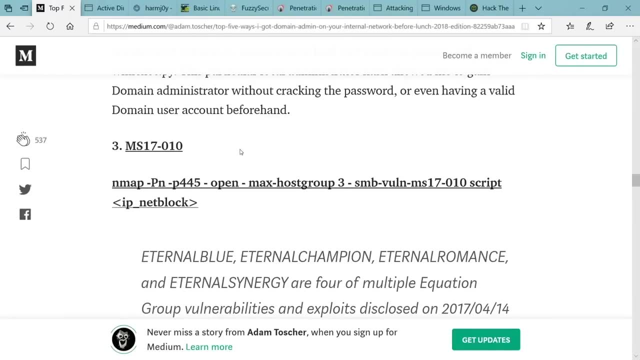 that we're going to relay to And if we keep scrolling through, what else has he gotten in here? MS 17 0 1 0 doesn't necessarily have to be an active directory environment, but you're going to find this. 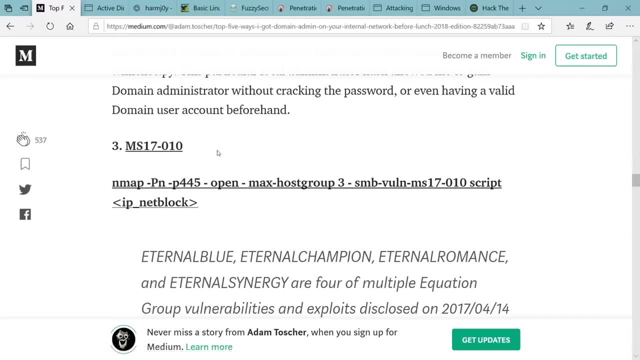 Hanging fruit all over the place. So there's not much to show or to teach here. but we do have a box- and I'll cover that in a minute here- uh, that we can cover with this via hack the box And uh. 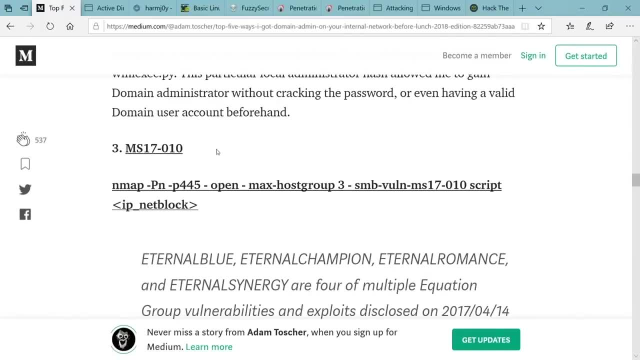 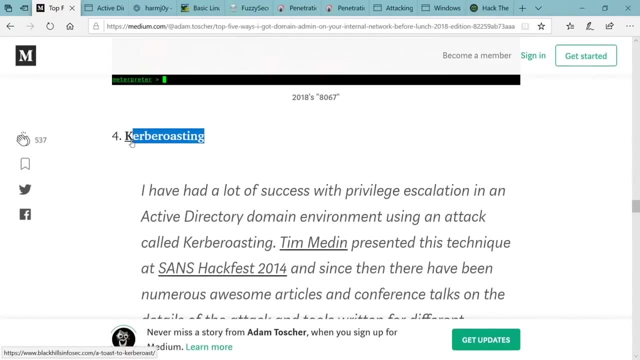 this is something that you should be looking for on every assessment. This low hanging fruit is is amazing. So also Kerber roasting. Kerber roasting is a big one. See it on a lot of assessments. And, uh, another box. 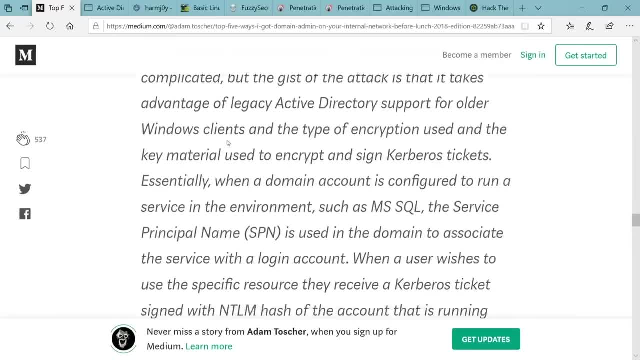 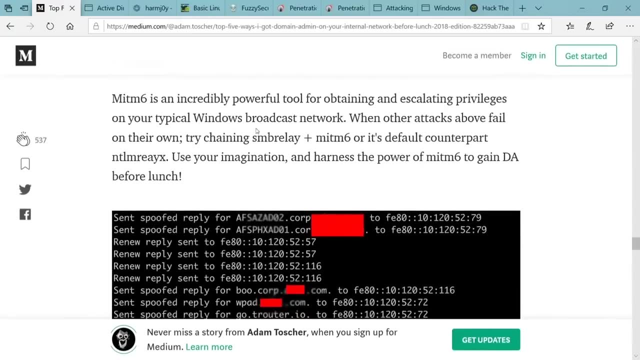 This is something that we can cover via, via, hack the box Again. we'll talk about that here in a minute, And I think MITM six- uh, this is the one that I use that much- uh, but something worth reading and looking at his tactics. I'm going to give you some extra homework tonight as well. 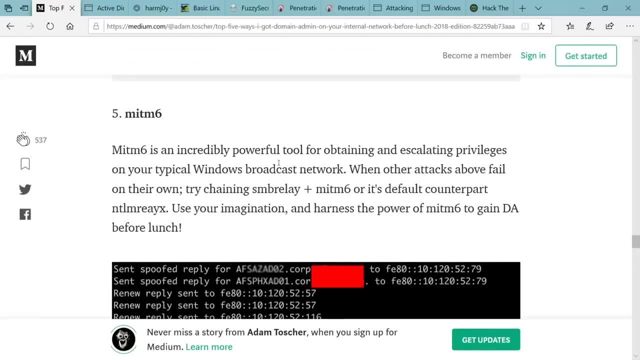 uh, when it comes to relaying and you'll, you're going to go on your own and do your own lab after what we've built out, And you can- uh, you can- go further with what we do, You're going to. 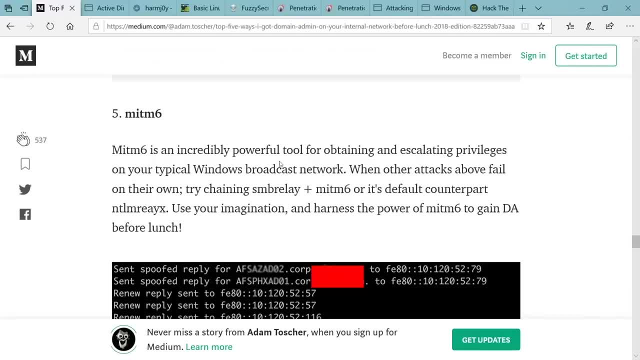 get a proof of concept tonight, And then I want you to take that further and explore what you can actually do with relay. Uh, I saw a sub come through. Thank you, Bammers, Brent, I appreciate that. All right back to our fun list. So on that list as well. 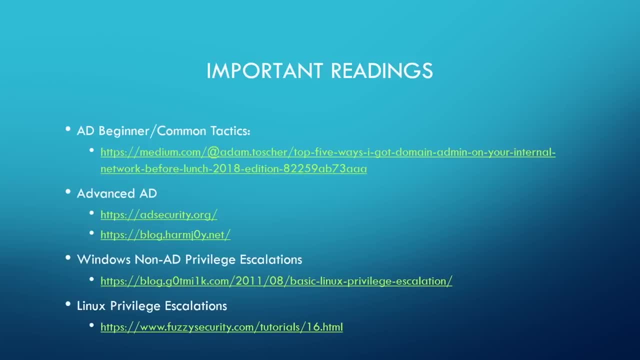 we've got advanced active directory topics. If you've never been to 80 securityorg or seem heart, seen harm joy's blog, you are missing out. Please do check those out. Uh, as well, we've got non 80 privilege escalations. 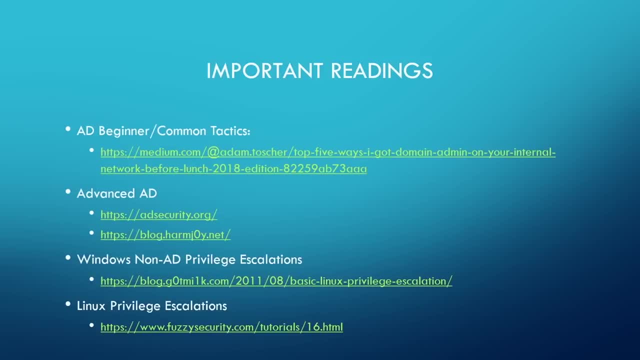 uh, windows version is got milk. Very, very good guide. I will be posting this and I can submit the links If you need to. please do take a picture, uh, if you need to as well, but I will be putting this on with the videos and Linux privilege escalations as well. These are: 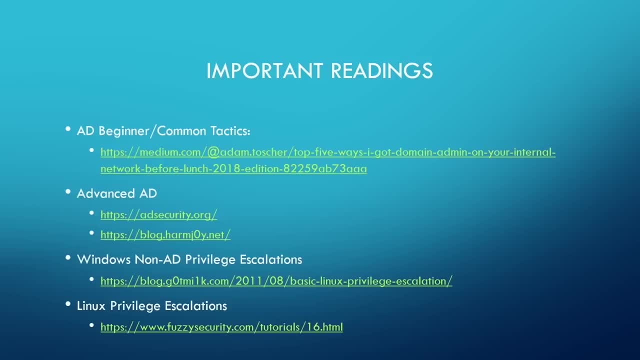 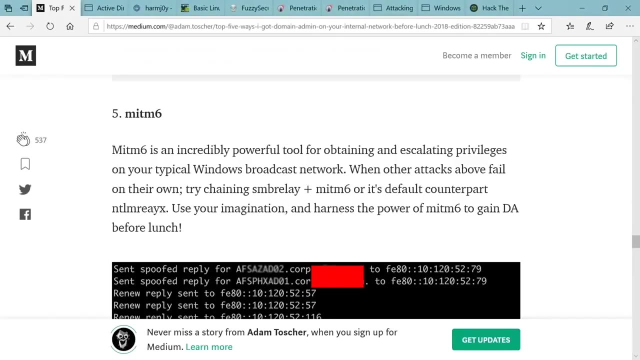 really really great, great blogs. So, uh, we can take a quick, quick look at those. And somebody asked why I'm using edge. I'm only using edge because I don't want to show you all my fun tabs, bookmarks and uh plugins that I use with Chrome and Firefox. 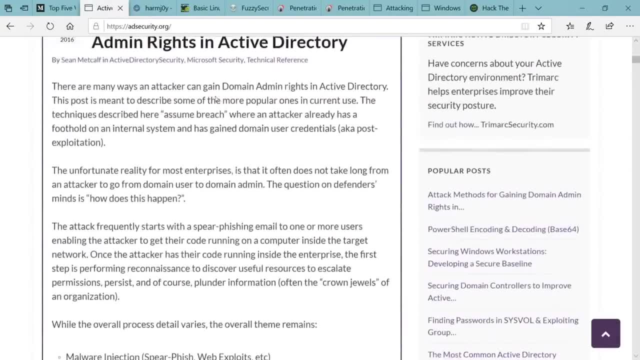 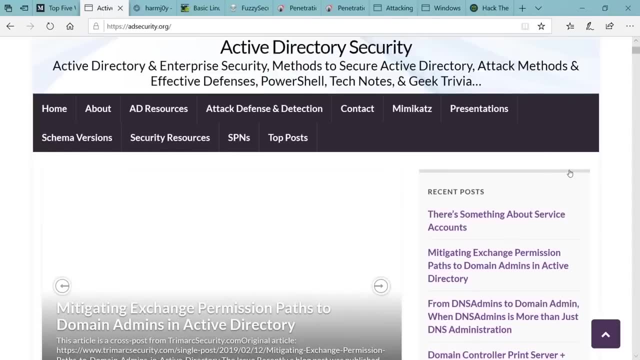 Uh, so 80 security. this is a Sean Metcalf website full of posts that are above my head, if I'm honest, but there's some really, really good stuff in here. uh, about learning active directory- Anything you want to know about active directory, attacks and security. 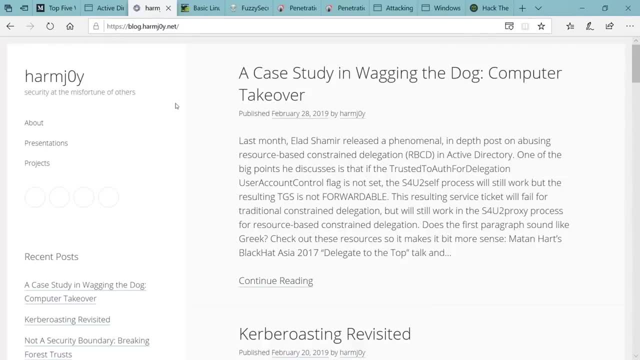 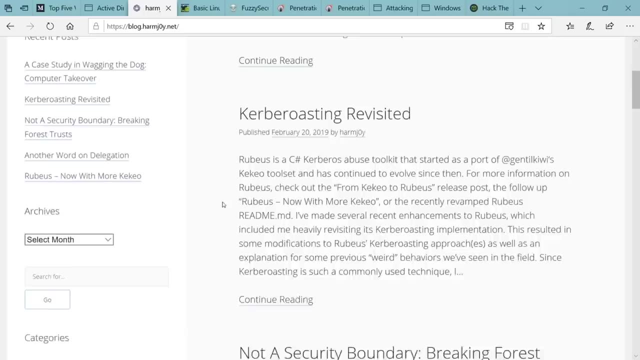 This is the website. I think harm joy is a close second. He does a lot with uh active directory attacks. He's got curb roasting in here as well. Uh, so worth a read If you want to go into some. 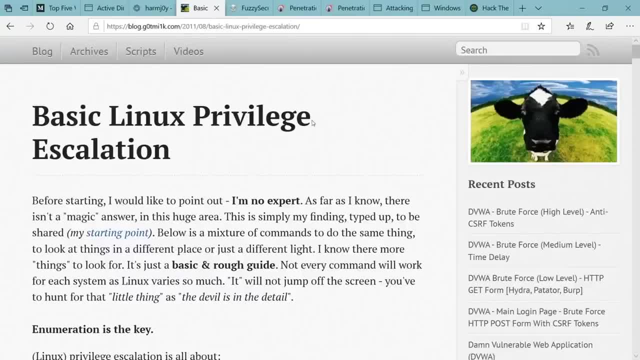 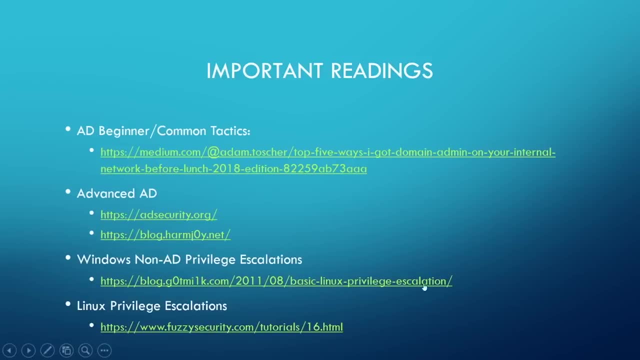 of this advanced stuff. Now, when we talk about the privilege escalation, we've got the got milk And I think I put this backwards. Uh, the got milk is actually the Linux And if I put that backwards, I'm sorry. I'm working on three hours of sleep tonight, So I did put it backwards, It's. 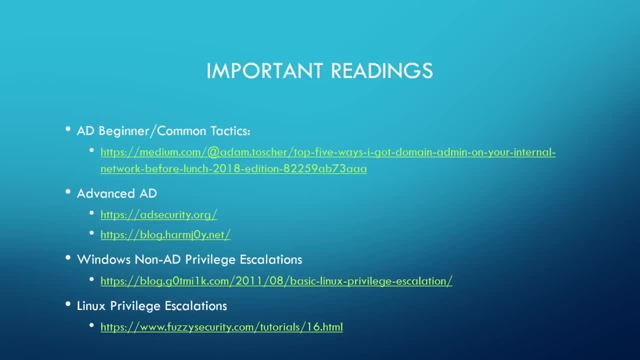 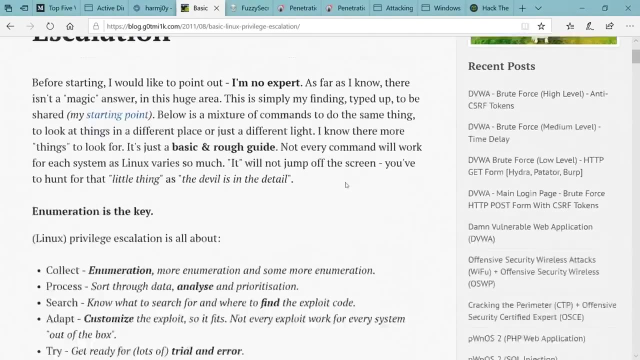 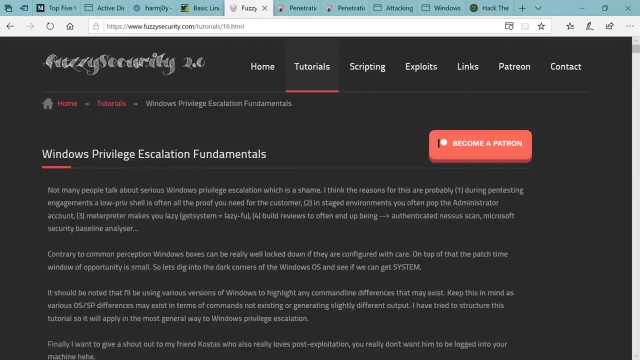 under windows, but truly it is actually Linux, and switch the Linux for the fuzzy security. Um, so this is the the God guide. you know, this is the Holy grail of Linux guides And this is the Holy grail of windows guides here for fuzzy security. So, uh, take a look at these. This. 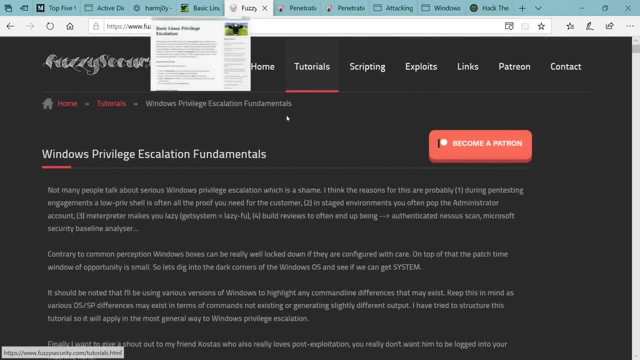 is more common and what you're going to see in capture the flag environments, the OSCP type stuff. Uh, when you talk about doing hack the box, any of those types of things, you kind of want to look at some of the common tools that are out there for these. uh, tools like like Sherlock or there's. 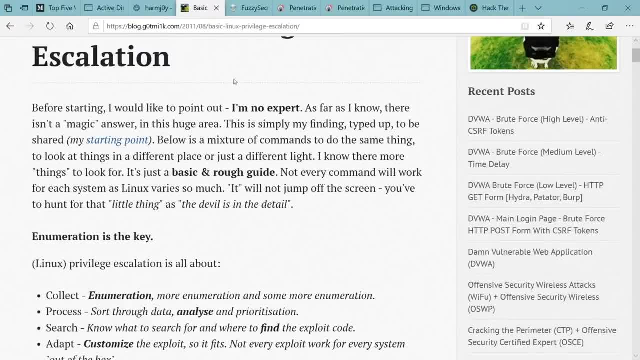 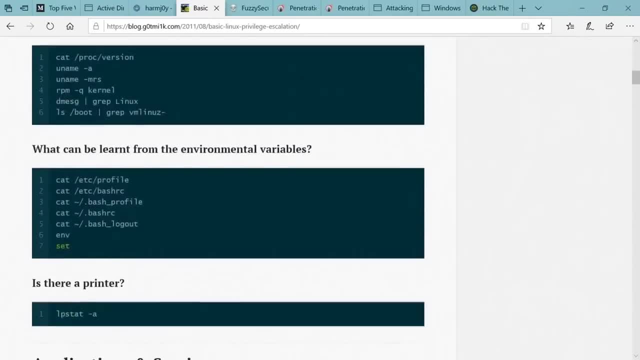 like the uh, the Lynn and Noomsh, or priv s checkerpi is another one for Linux. Um, so some of these common tools that can do some of this automatically for you, and look for some of these, and we're going to talk about the meterpreter version of that tonight, once we get into it. 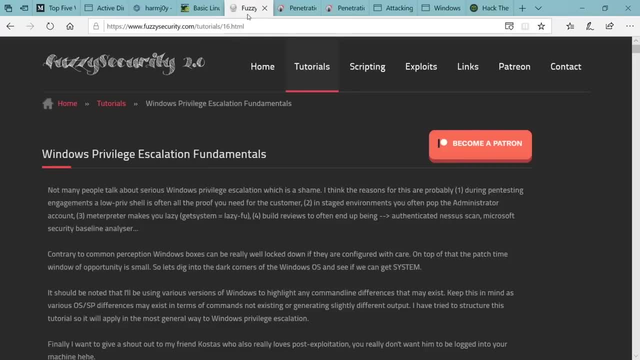 Uh, but also just note both of these blogs and, and if you ever pursue, you know, or do hack the box, keep these in your back pocket as something to have for research. All right, So we've got a bunch of questions coming through. Uh, let's see, Should we? 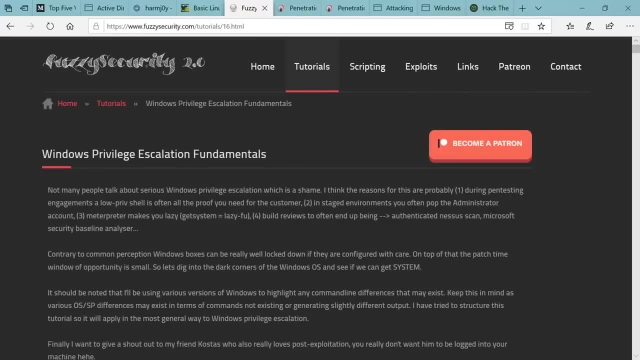 domain join the fourth machine? You can if you want to get ahead of me, but I'm going to be showing it. Do I share the presentation? I can share the presentation. I will be sharing the links in the discord channel and I will be sharing the links on the YouTube. So 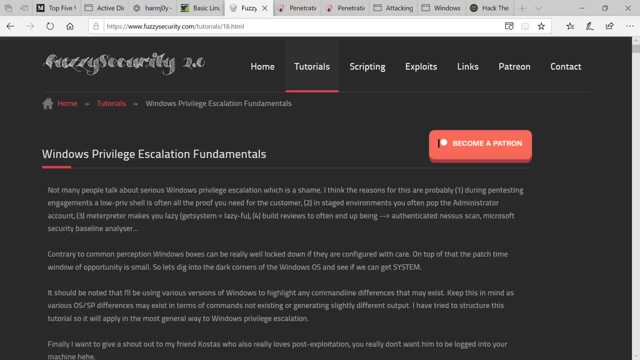 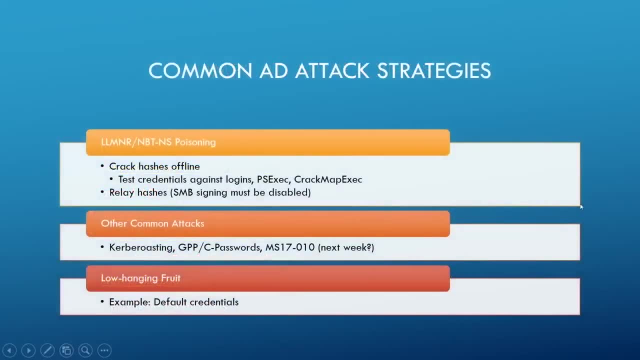 okay, Back to our presentation. So let's look at some common AD attack strategies, Most of these which you just saw. So we have LLM and R, MBT and S poisoning. We started that. last week We cracked our hash offline. Now we are going to see what we can do with these hashes, these offline. 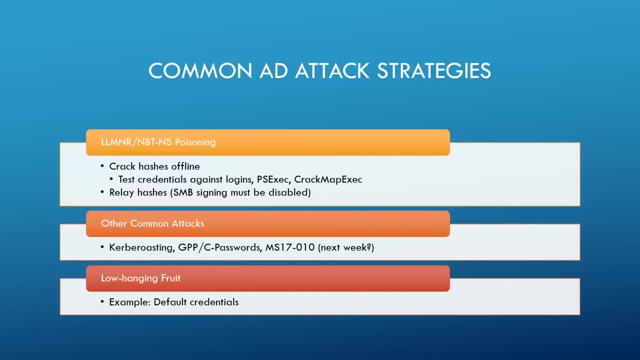 cracked hashes, Uh. so we're going to test the credentials against logins. What I mean by that is typically we're going to look for, you know, SMB and we're going to use PS exec for that or crap. crack map exec with that, Uh. but you know, any 80 login will work. You check on any web pages. 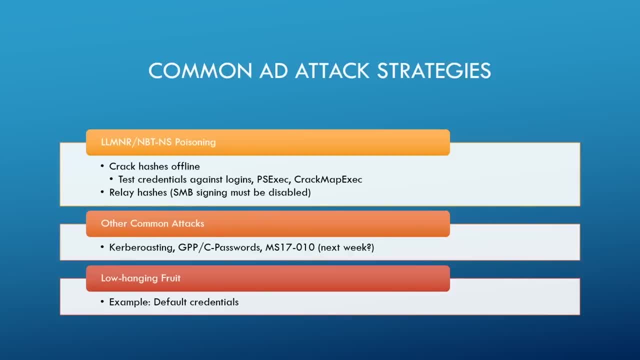 that are out there that might be using active directory and allow you to log in. You never know what you might find on top of that. tonight we're going to be talking about relaying hashes, So SMB signing must be disabled for this, And by default in most environments, SMB signing is. 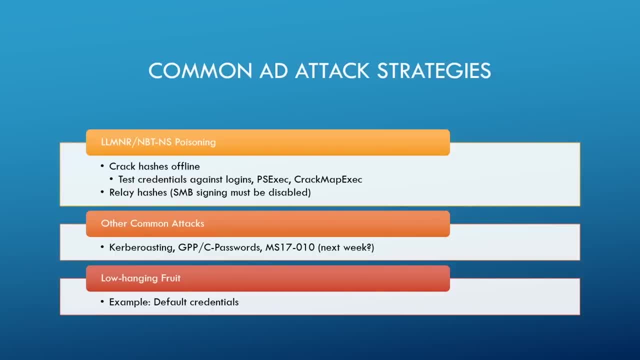 disabled And a lot of admins don't like to enable it because it causes issues with speed. Uh, so you'll find SMB signing turned off most of the time. We're going to go in and make sure that it's turned off in our settings. 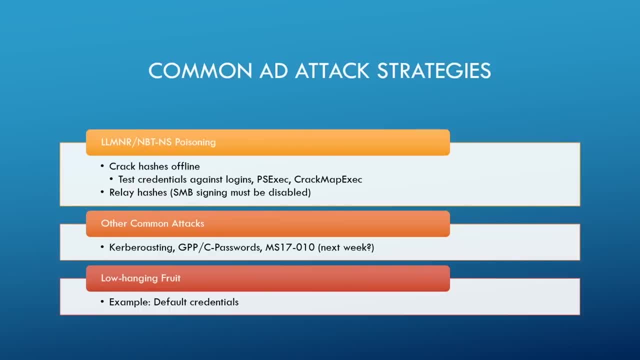 tonight, So you'll get to see where you turn it on and turn it off from from a defensive perspective. Uh, some other common attacks. We talked about Kerberosting, the GPP C passwords and the MS 17 0, 1, 0.. All of those can be taught. next week We're also going to be covering 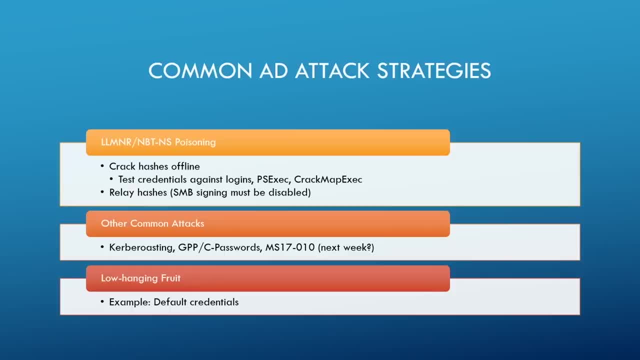 token impersonation. tonight I've got quite a bit I want to show you guys, uh, depending on our time limit, So uh, and then also some things to look out for is just low hanging fruit. So an example of that is default credentials, And I've told this story before, but I've told it in. 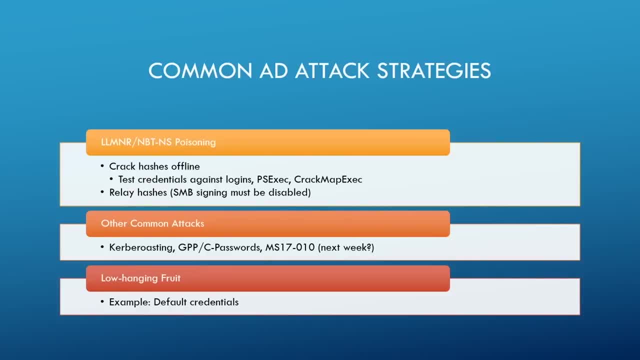 the Q and a usually um one of my favorite assessments that I've ever had: I got domain administrator off of default credentials on a printer, So you have full potential to find domain admin in the weirdest possible ways. Uh, so just because 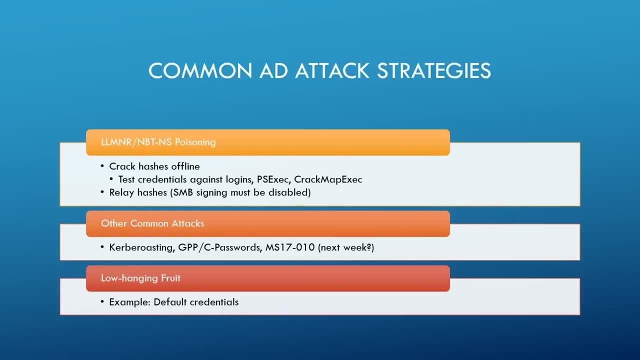 there are no you're. you're sitting there with responder, You're not cracking any hashes. You're finding that everything's patched Doesn't mean that there's not something out there that is improperly configured or misconfigured and allows you to gain access. So always look for the low. 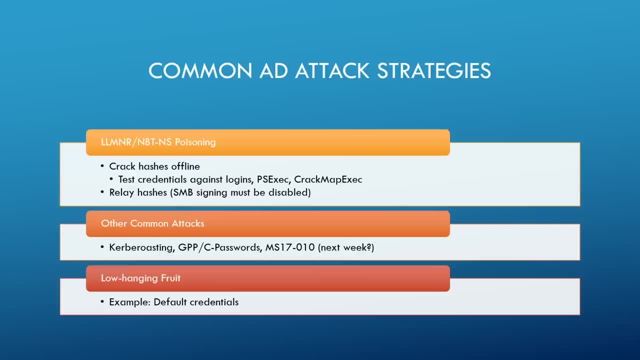 hanging fruit- You never know what you're going to uncover- And to go into the other common attacks and the ones that I want to show you. So let me go back and we're going to be on hack the box a couple of times. So if we come on to hack the box here, 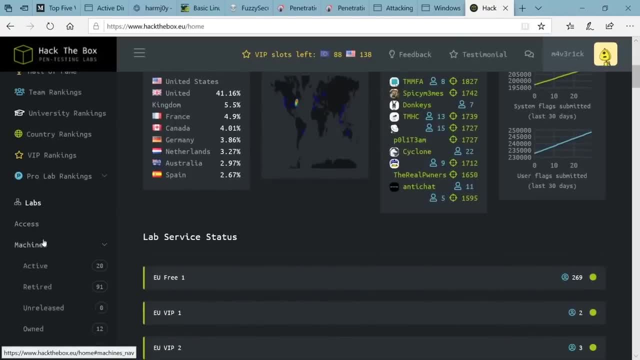 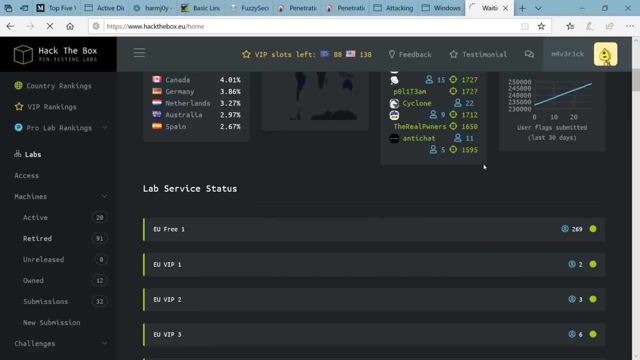 and you have a VIP membership. come down to machines, come down to retired May. take a second to load And I have full faith that active is going to get voted in. It's already got a lot of votes, So if you want, please direct your vote to active And I have full faith that. 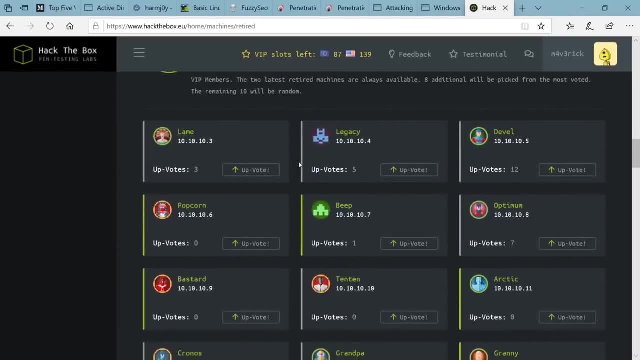 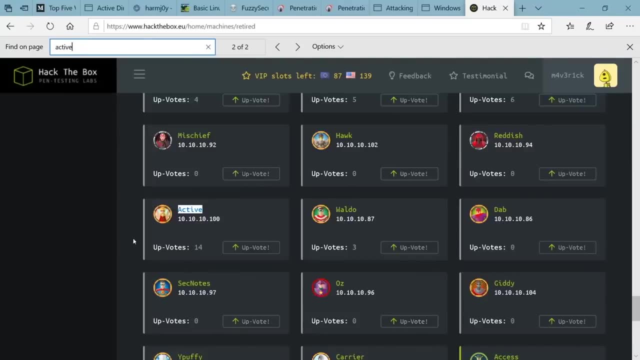 active is going to direct your votes towards blue. Uh, cause that'll allow us to have a little bit more flexibility. But if you search active, active has 14 votes. It's killing it this week. Uh, let's check in on blue. Blue's got three votes. Blue needs some love. 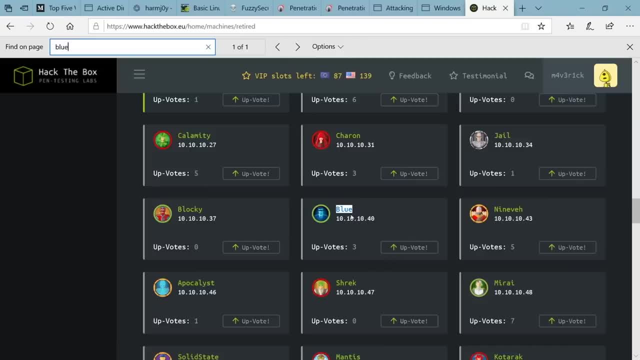 So I mean, blue is going to be a box that takes us probably 15 minutes to go through, Um, and you know it's not going to be that exciting, but it's still going to be a lesson for people who are new and to understand what's going on. So if you're looking for a box, that's. 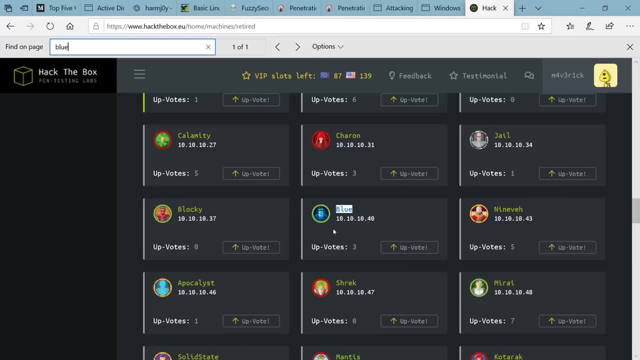 going to help you understand. uh, you know the MS 17 0 1 0 exploit, So I'd love to show you those two and maybe even get through the end of the course next week, And we may just do a special. 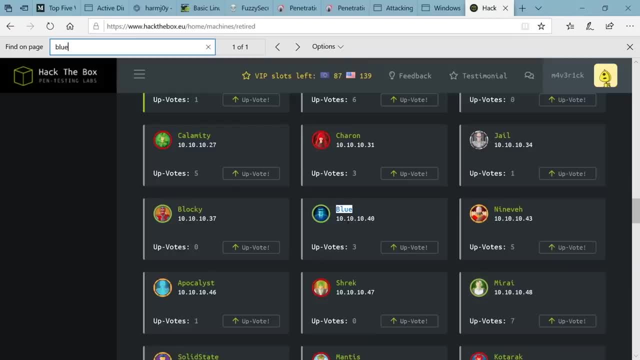 capstone. Now that I'm thinking about it, I may give you guys a capstone, uh, in the final, final week of May, So on the 28th. what we'll do is we'll just take some of these old boxes. 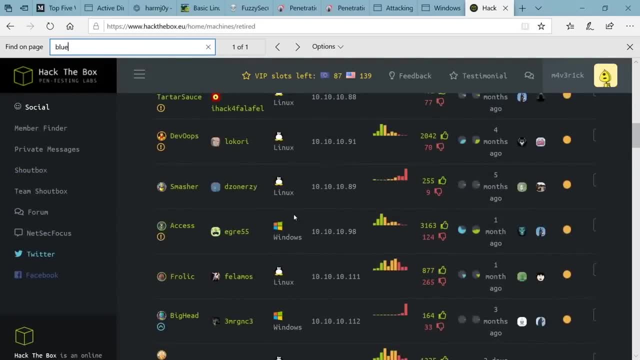 and I'll walk you through the process of how I would enumerate it, how I would attack it And I would try to pick the most realistic things. So you can see it from a penetration testing perspective, from enumeration perspective, and we can kind of start it from start to finish. 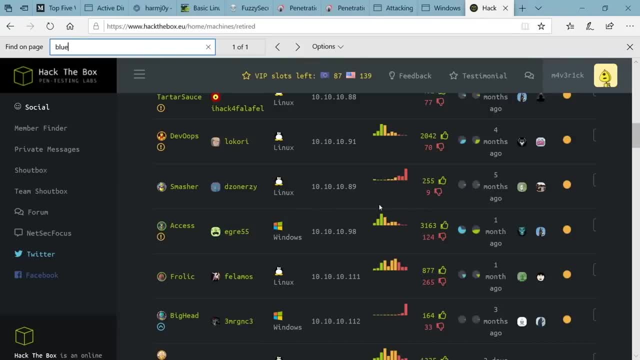 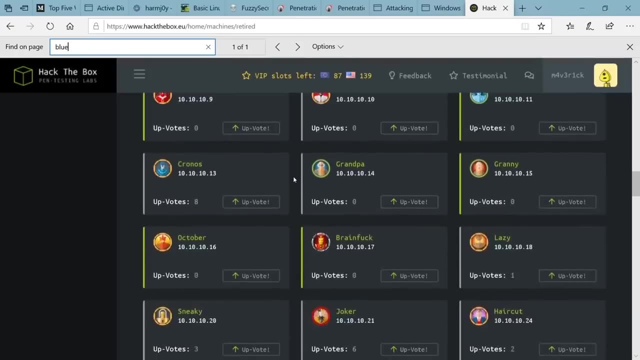 and see how I would attack in my perspective. So, uh, please do upvote these if you can, if you'd like another week, if you don't want another week with me, that's fine as well, We can. uh, we can end early. So, with that being said, let's go back to the slides one more time. 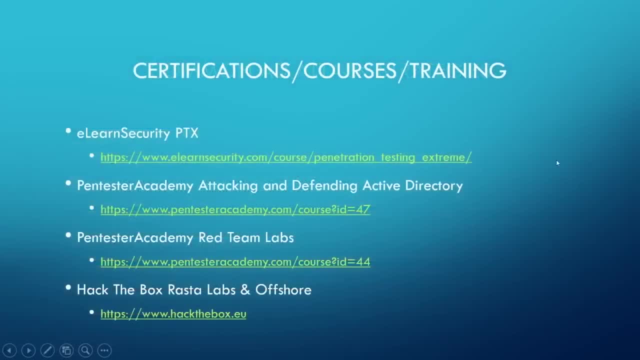 And let's talk about certifications, courses and training. So I'm going to repeat that what you're learning for me is the beginner, the basics, everything you need to know. I'm not going to be able to teach you- I could do this for weeks. Now there are some great courses that. 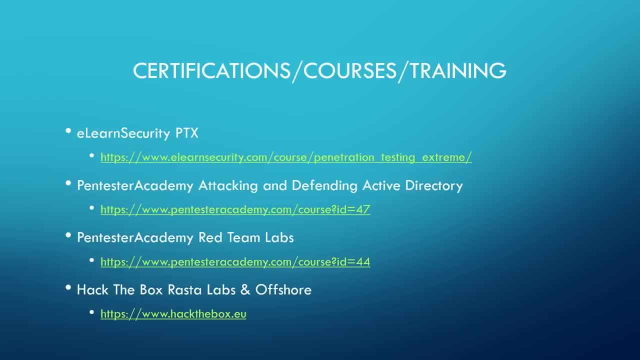 are out there that can teach you some more advanced AD tactics. I've already provided some blogs for you, but if you're a certification, video, training lab kind of person, there's quite a few of those as well. So I'm going to start with the basics. So I'm going to start with the 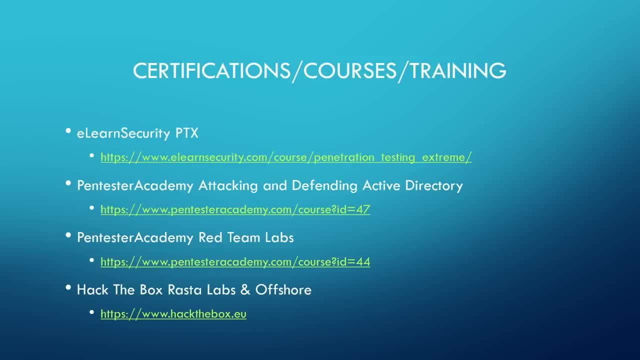 so first one I'd like to show you is the e-learn security PTX. I've heard mixed reviews about it. I actually have purchased this and I haven't gone through it yet, so I cannot confirm or deny how those reviews are. Um, but I have heard that it goes kind of well with uh, hack the box. 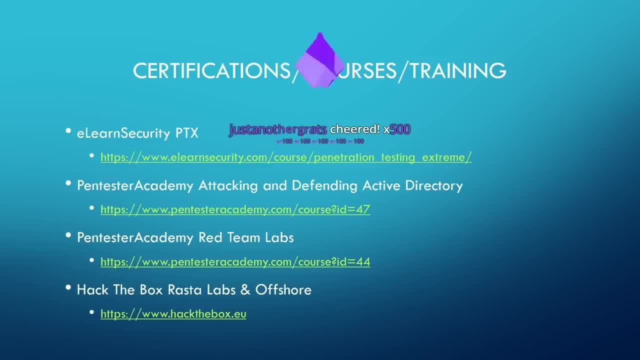 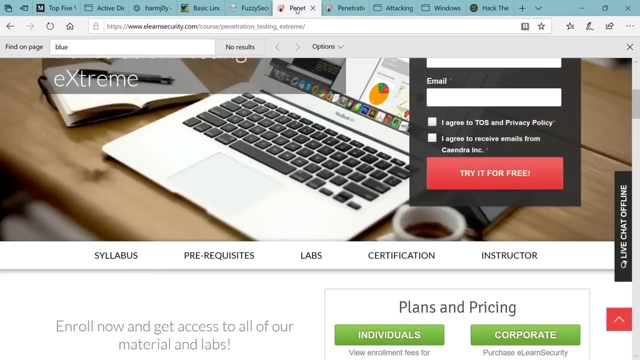 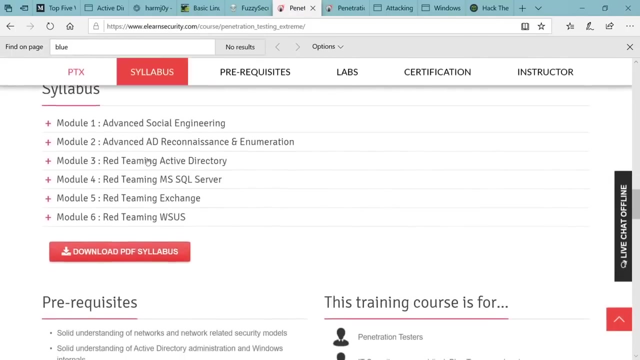 the pro labs which we'll get into here in a second. So if we look at it- Hey, thanks, Gratz, I appreciate that. So if we look at it here, the PTX penetration testing extreme- it goes into advanced tactics. It's got social engineering. 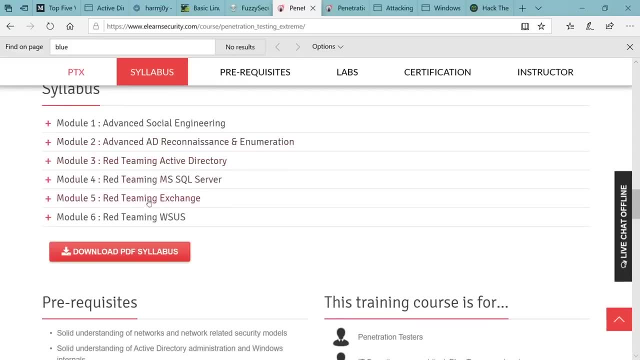 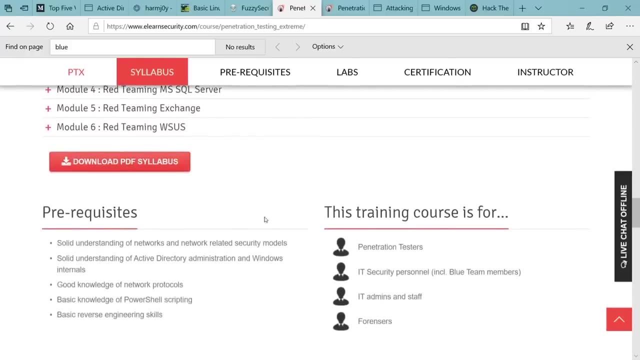 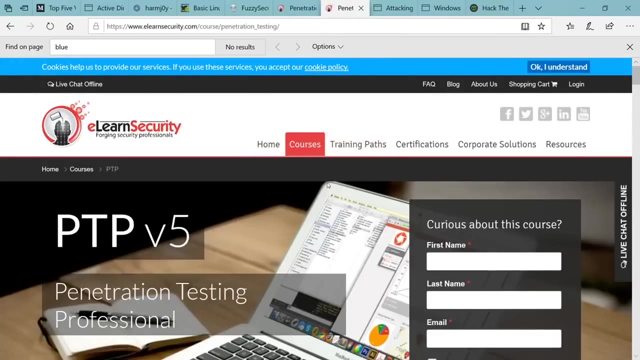 uh AD reconnaissance, red teaming, active directory, red teaming, SQL server exchange and uh WSUS there. So, um, some things to look at, but a a good shout out goes to actually PTP, which is kind of the competitor to the OSCP. A big shout out here because if we 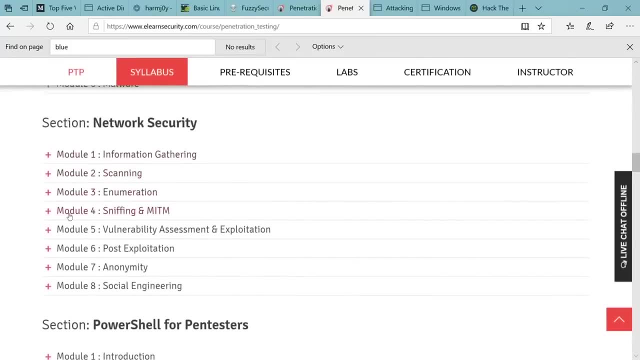 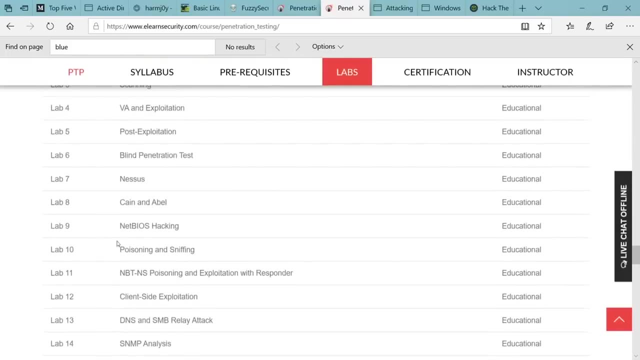 scroll down into. let's see if it's uh sniffing man in the middle. Let's see if the labs are hold on. I know it's in here somewhere. If you look at lab nine or actually, sorry, lab 11,, they do have MBTNS. 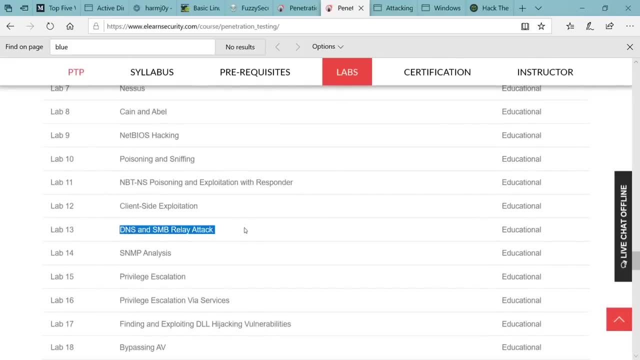 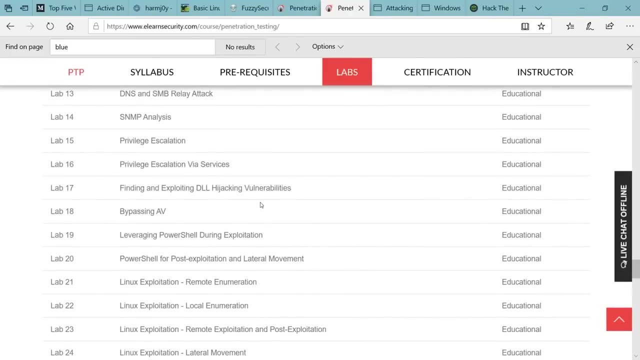 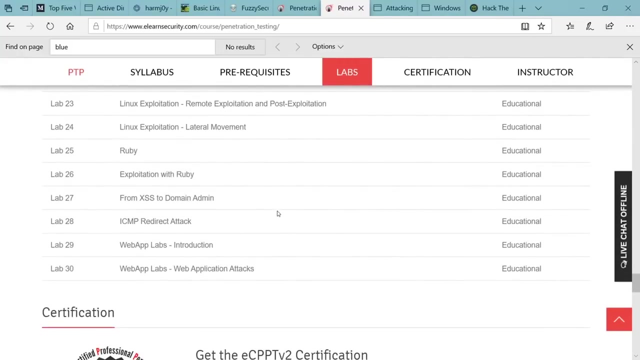 poisoning exploitation with responder: Uh, they've got DNS and SMB relay attacks. They've got different types of privilege escalation, bypassing AV, et cetera. So, um, this here. this here is why I have been so uh adamant about eLearn security and why I say: you know like, 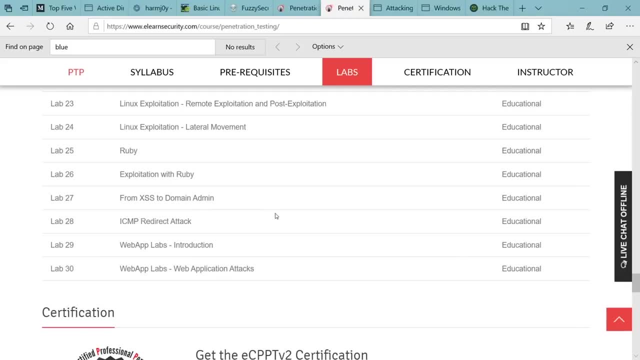 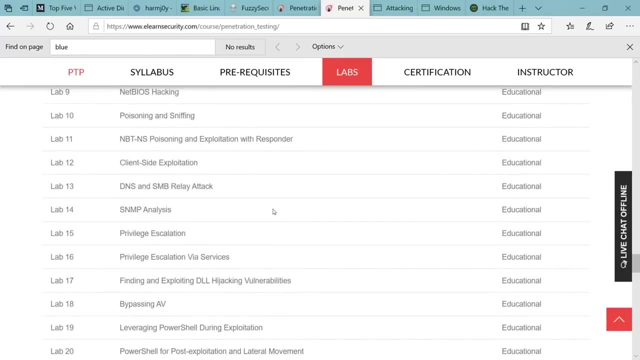 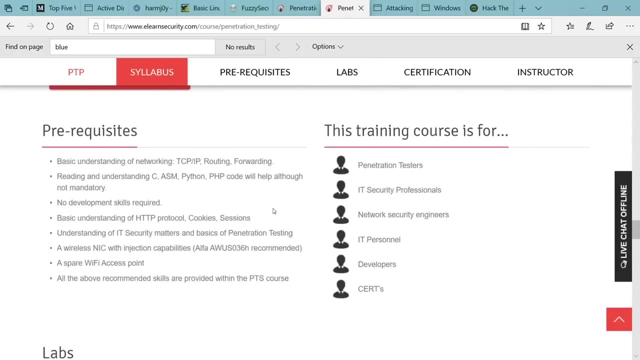 PTP is really out there because, like, if you're seeing the attacks that I'm teaching you, they're really upping their game in terms of being relevant and staying with the times. they update within every three years. Uh, this is great, great stuff, So worth checking out. I. 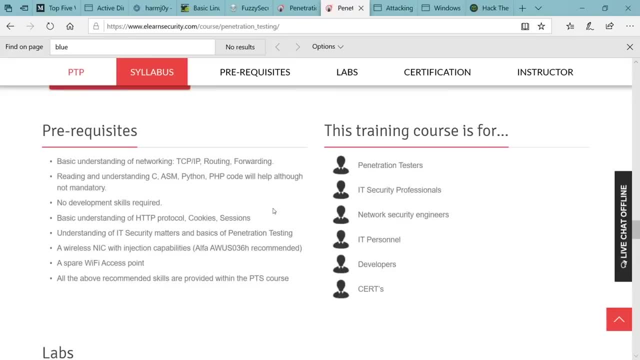 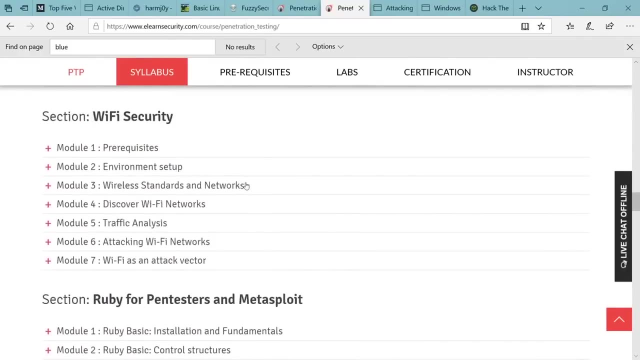 like I said, I don't know about the PTX. I have not taken it yet. It's on my list. I do Um, but it's definitely worth looking through this and it even teaches you things like wireless and programming. uh, you know some web apps, So it's really cool that it goes over. 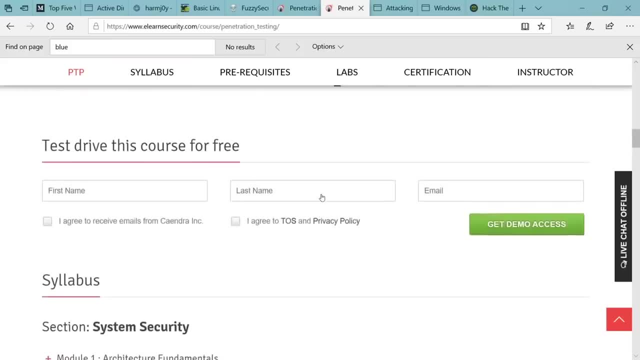 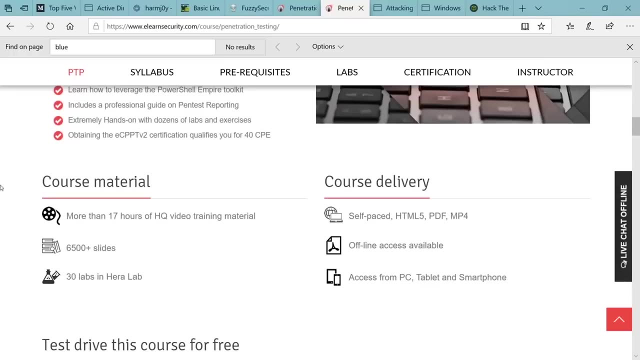 all these, these tactics from a broad perspective, Um, so worth looking into and worth, uh, you know, purchasing if you have the, the funds and the time to study it. So somebody said their interface is nice too. Their interface is really nice, Very, very nice. 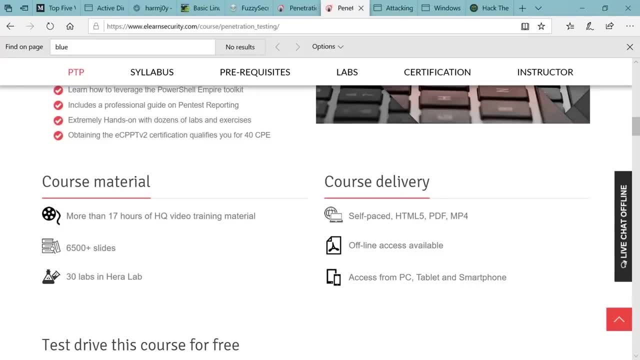 Okay, Would I recommend taking this after the OCP? Yeah, I think it would still give you a leg up, because the OCP doesn't have nearly any of this. Can I send the slides on the discord? Yes, Yes, I've mentioned that. I will send the slides on the discord. Uh, do I recommend sand stuff? We're. 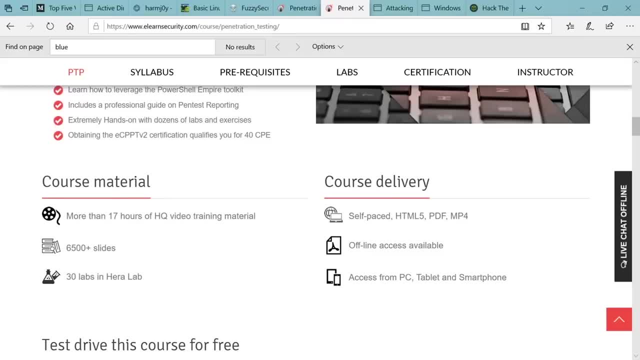 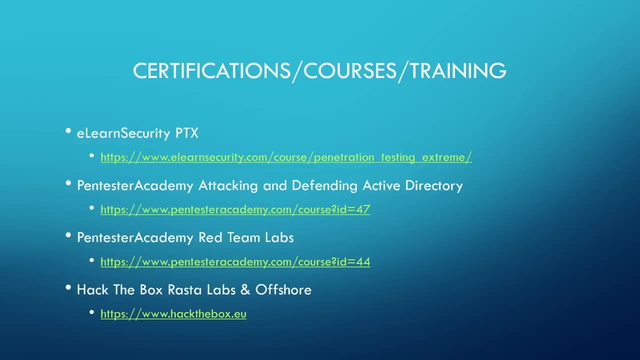 going to save the questions for Q and a guys Q and a time afterwards. So, all right, let's go into some other resources here. So there's two pen tester Academy resources. I'm hearing good things, The attacking and defending active directory. I actually purchased this and I'm in the labs now. so far, So good. I think that 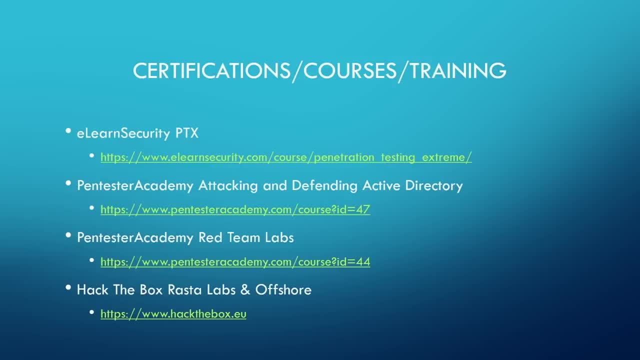 it's actually a really good course. Um, the advanced version of that is the red team labs, and I have both of those brought up here, Uh, so I would start out with, uh, the attacking and defending active directory and then moving on to the red team labs. Now, neither of these will. 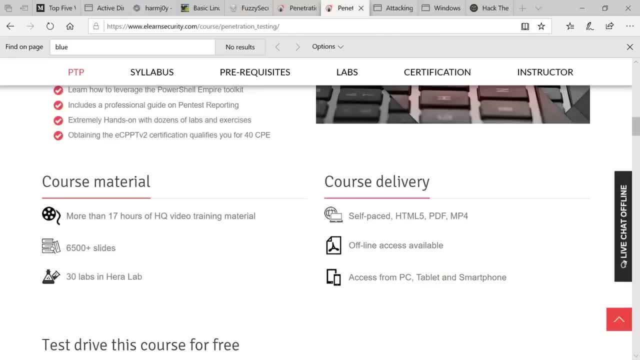 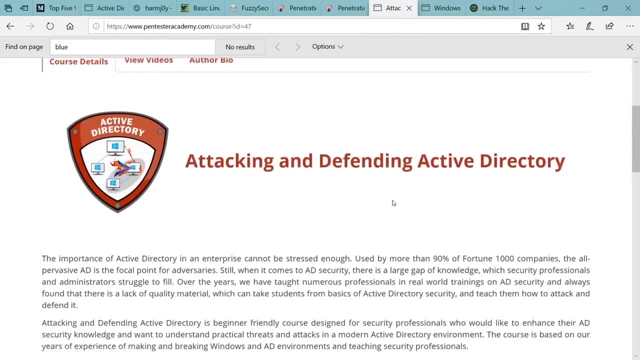 give you a certification that is HR worthy. If you're after it, you're going to get a certification for the HR. You're in it for the wrong reasons. Same thing with eLearn security. These are for pure knowledge based- uh learning. There's the certifications. really, just don't. don't do it for. 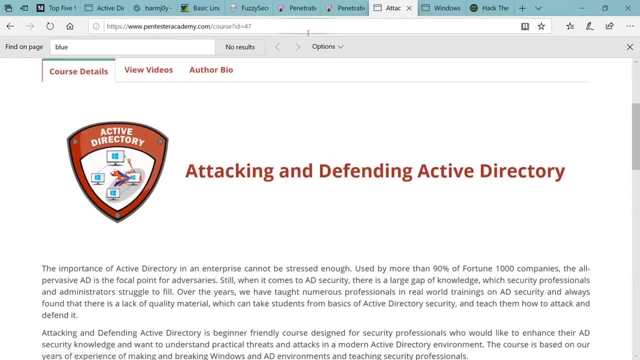 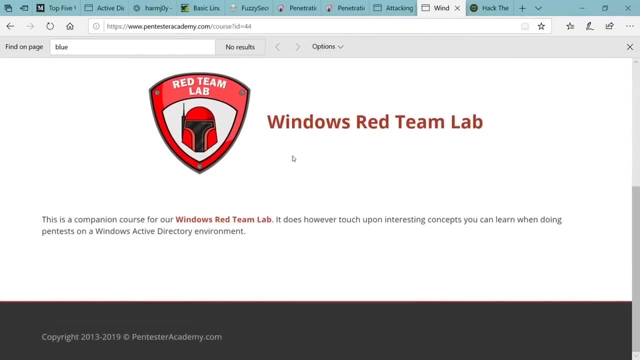 the HR. Um, so you've got this course here, attacking and defending active directory. Like I said, that's more of the beginner course. And then the red team labs are there. Uh, they're more intense course and it's focused purely on hacking active directory. 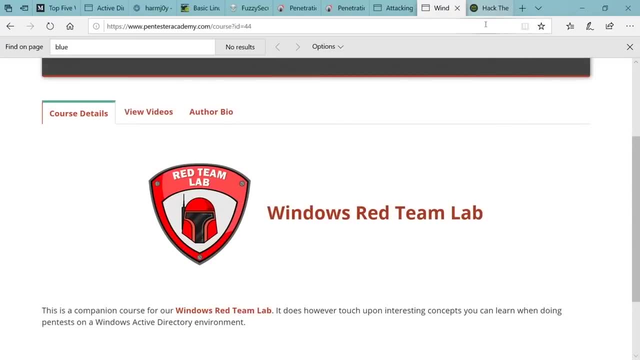 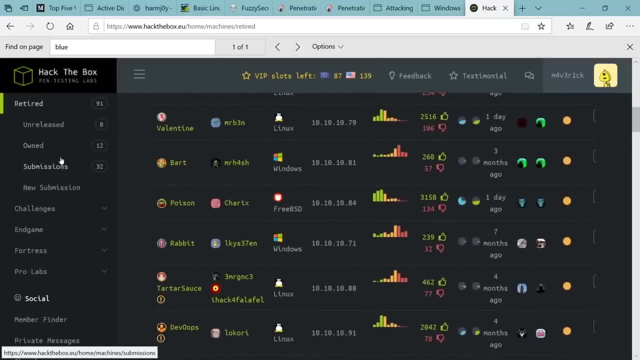 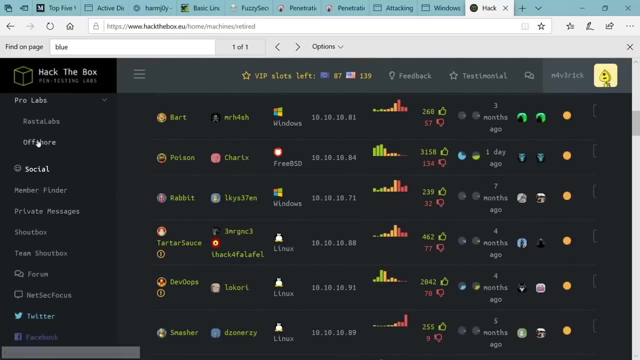 So, last thing, and I'll just skip the slide and go right to hack the box. Hack the box has two pro labs. Now. these are probably the cheapest solution out of everything that I've shown you, but this is going to be most of your, of your research. time is going to go into this If you come on. 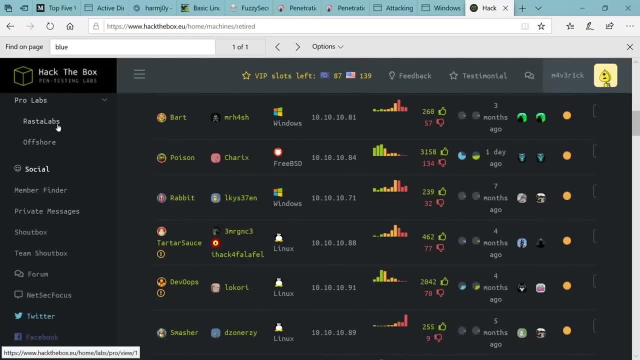 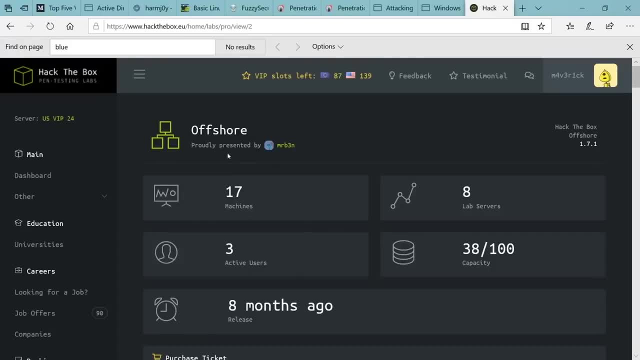 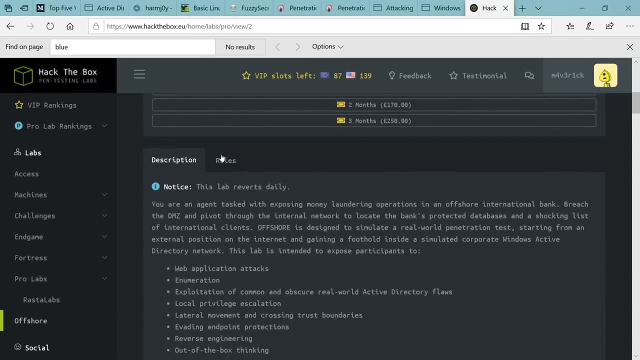 guy and a big time Vous Creating Commenter And you know, one of the things that was really interesting to me was Ben petites is an actual pentest that he went through En. I've heard nothing but good reviews about it, So it really emulates what a active directory environment is, And a pentest. 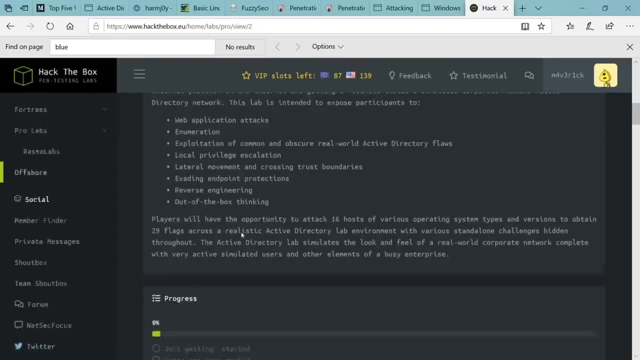 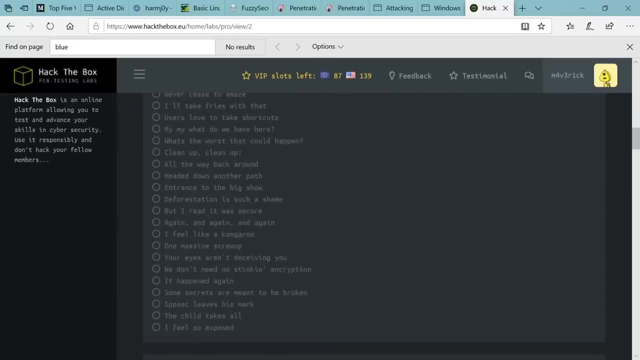 is like for one of these And, uh, you know, just has some some crazy outside the box tactics that you really need to to learn. En, it's got all this checklists in here that you need to go through. So, um, very, very good environment from everything I've heard And it 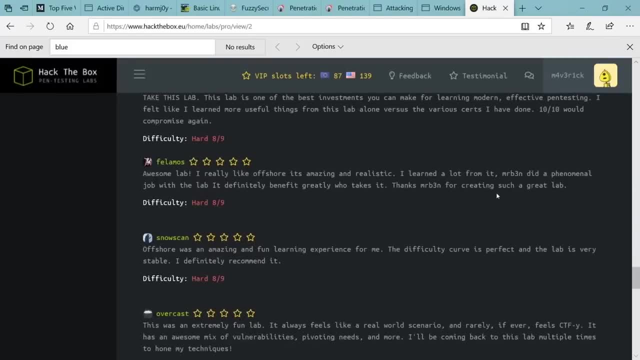 will to a lot of things, Even at 8%. I and aра, I think he's, I think Ben btests in puts and it really does. If you just edit Welt FIFA, I've heard, and it will challenge you. so, with that being said, these are your options. please do look. 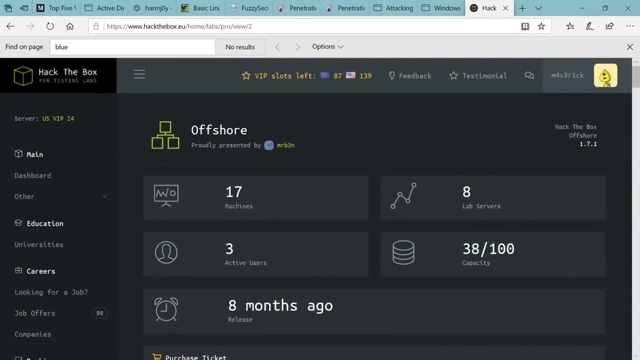 into them. I'll bring up the slide one more time so you guys can take a picture. as I've stated, I will send these slides out in the discord channel and I will be posting the links down in the description on the youtubes. so here is the slide one more time. I'm going to grab a drink. 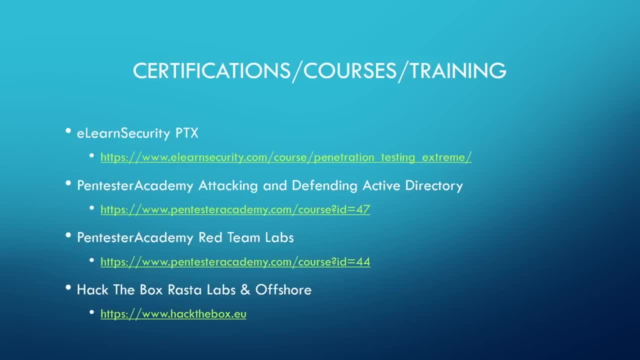 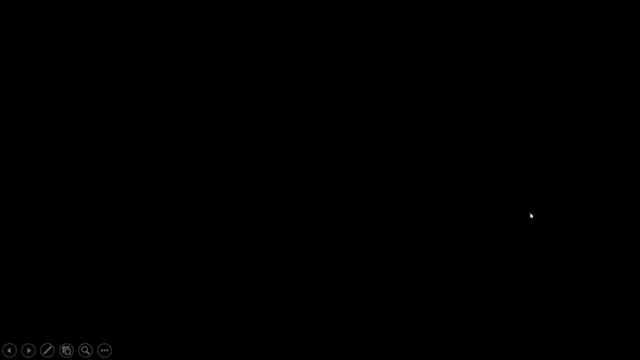 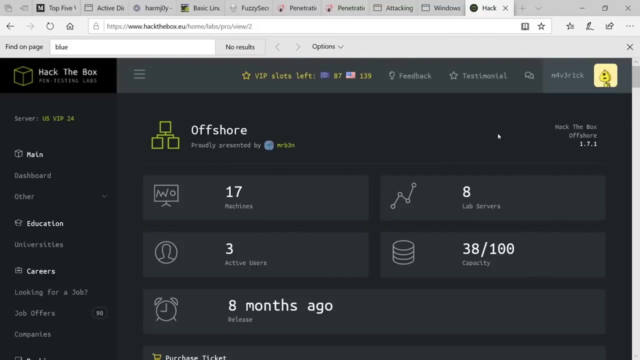 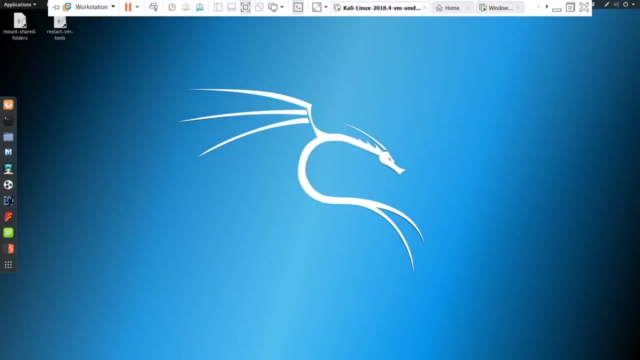 all right. so that is it for the powerpoint. I'm done boring you guys with that. it's rostlas made by rastamouse. it sure is all right. so where did we leave off last week? we left off capturing the hash of the punisher right. 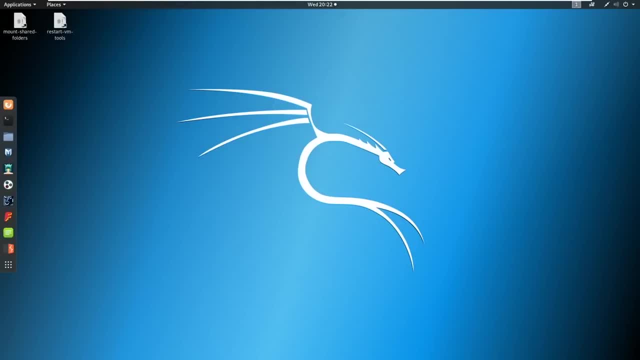 we left off capturing the hash of the punisher right. we left off capturing the hash of the punisher right. we captured his hash, we went and cracked it and we we realized that his password was password. one with a capital p didn't have the greatest of security, so we're going to run a. 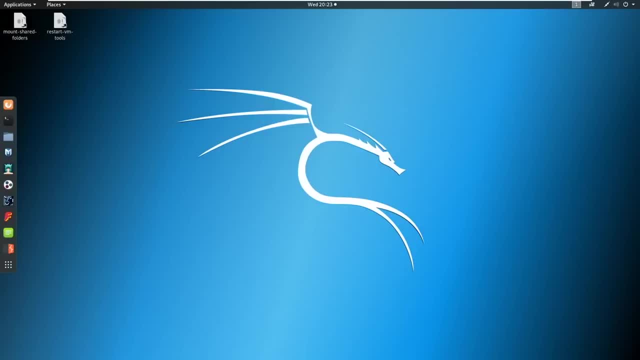 scenario tonight, something that we see quite often when it comes to pen testing- and that is a situation where we leverage those credentials into getting- uh, getting domain administrator. so we're going to need to do a few things. so, again, we have our cali machine, we have our windows server here. we're just going to 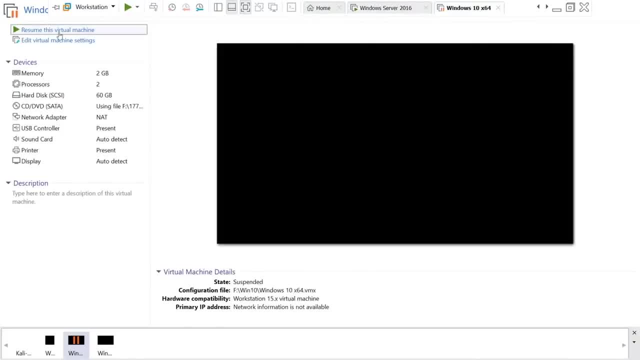 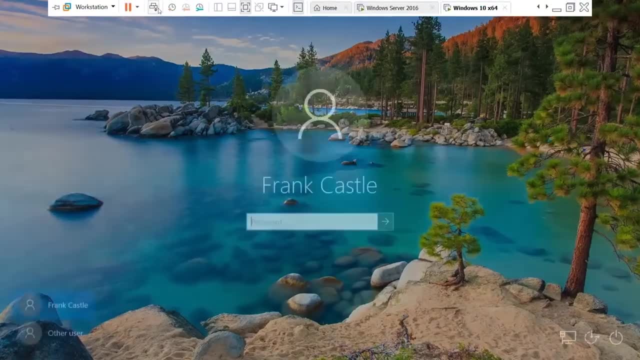 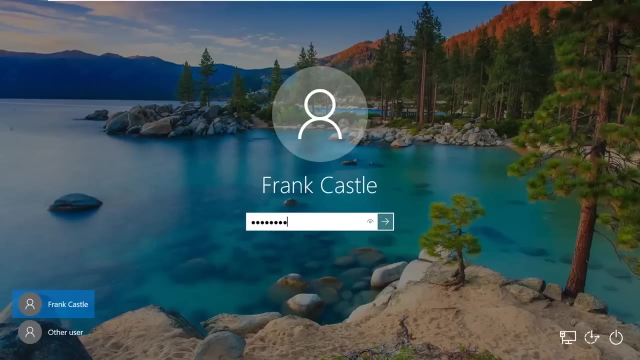 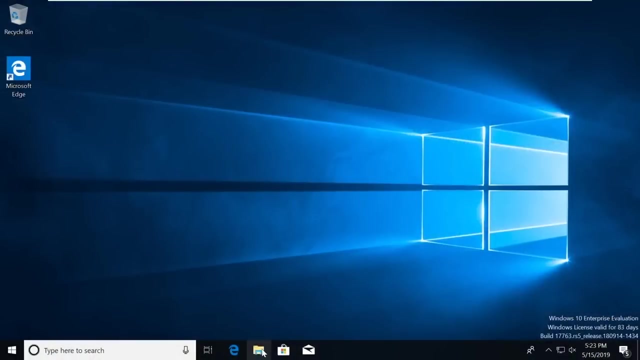 let that sleep, and then we have our windows 10 machine from last time. let's just go ahead and power this on if yours already isn't. let's get logged in here. let's go ahead and power this on, if yours already isn't. okay, so if we come into the c drive, 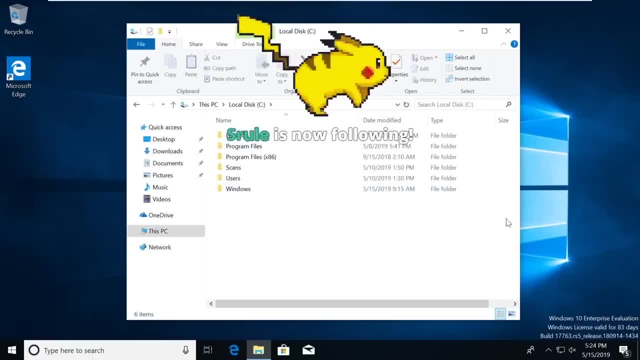 i've created a folder here because i was doing testing for this lab, but i'm going to have you guys recreate everything i've already done and i will stall chat, do whatever, so you guys can catch up. so please do create a scans folder. this is emulating something i have already done and i'm 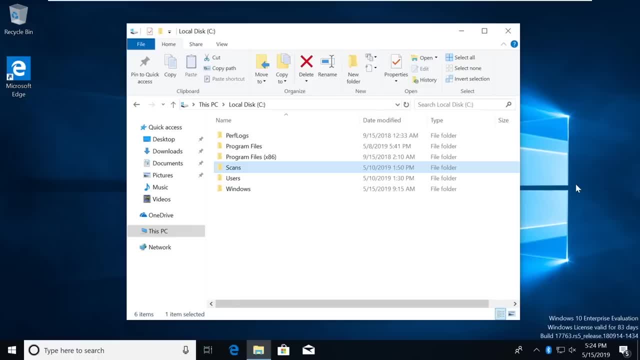 going to create a folder that you can see in a real life environment, plus some other situations that we're going to see now. commonly users have a scans folder located somewhere on their computer. it's got a user scanning to it or their own account scanning to it. 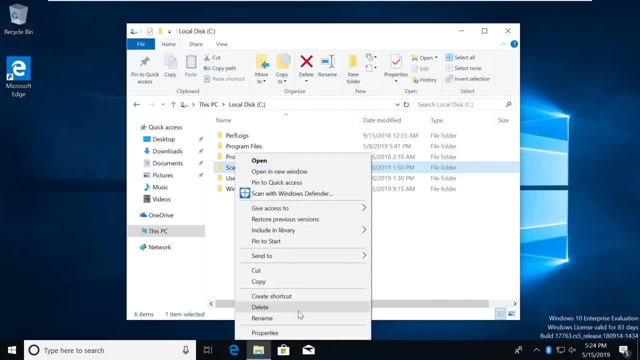 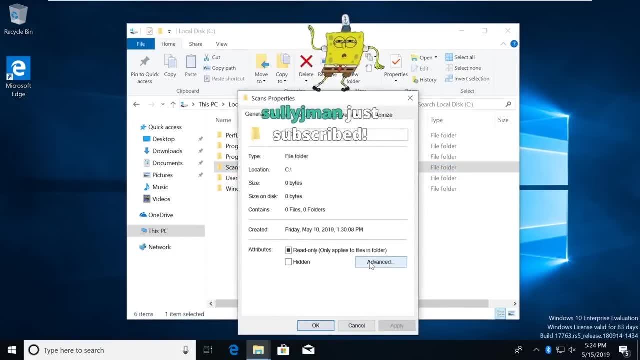 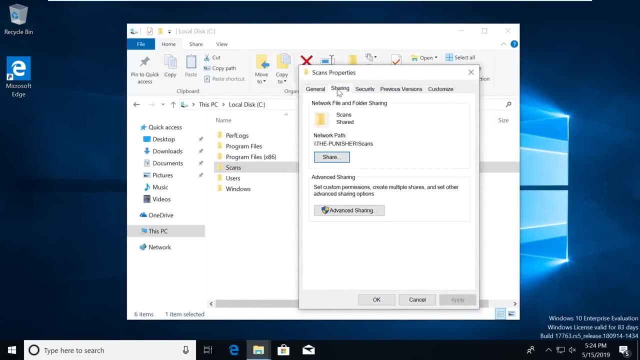 so what we're going to do with that is we need to share that folder out so that the folder has smb access and can be accessed by the printer or whoever it is that needs to access this folder. so you're going to right click click on properties, go to sharing, and you're going to hit share and the settings I have for 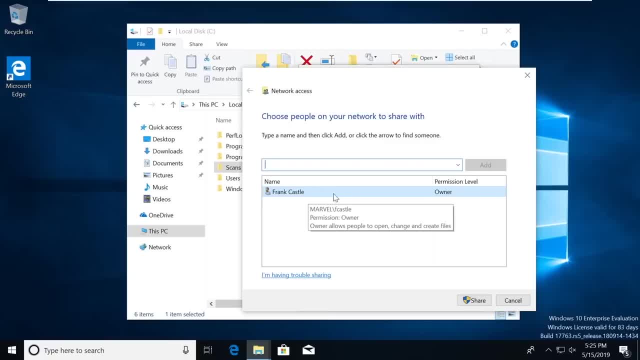 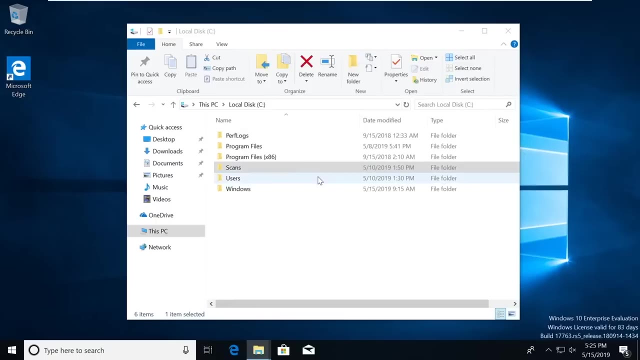 this is. I'm just sharing it with the owner, Frank Castle. it should be your Marvel Frank Castle account, or whoever it is that's tied to your domain. so hit share done. now, if you, you may notice that he is a local administrator for me. I've already made him a local administrator, we're. 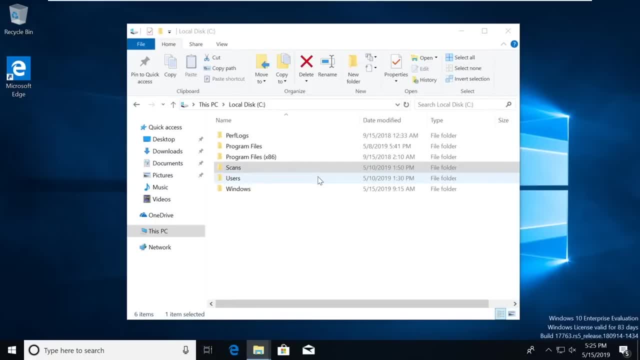 going to do that in a second, but you may need to enter credentials in for your administrator. hopefully you remember those from last week. but once you have that shared out, we're going to go ahead and make good old Frank a local administrator for this machine. this is also very, very common. 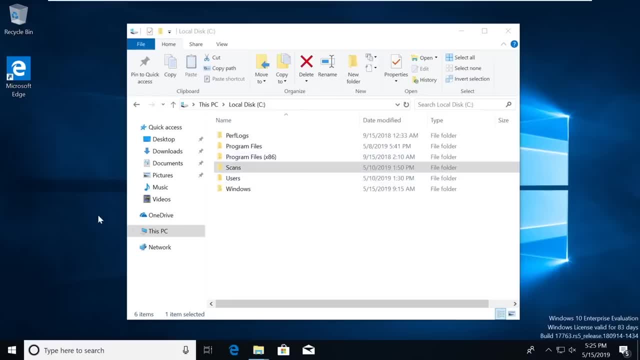 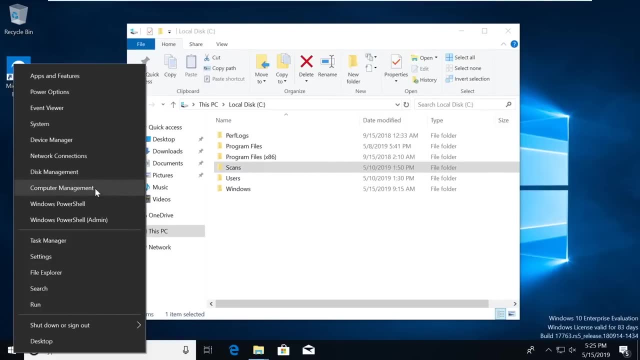 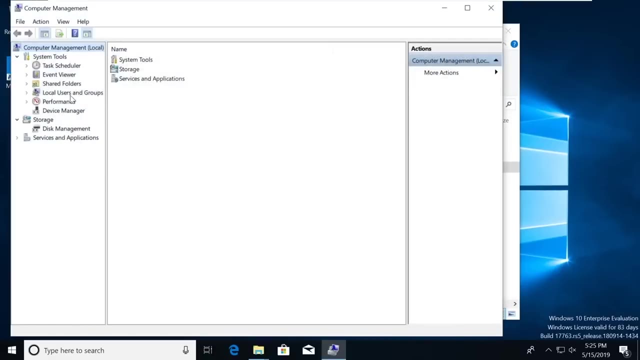 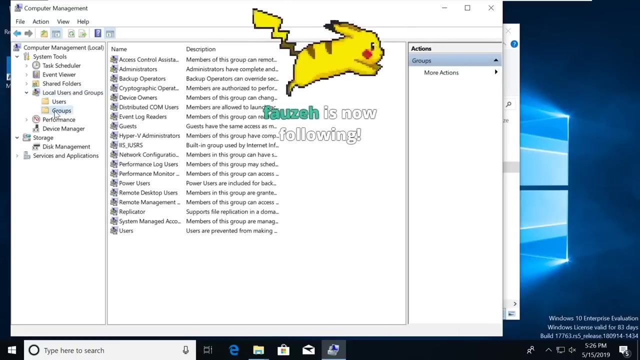 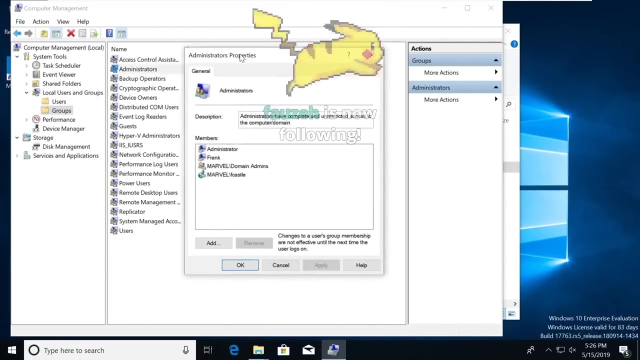 in in environments, working environments. so let's go ahead and just right click on the start menu and we're going to say computer management, we're going to click on local users and groups and we're going to click on groups. now, from here, we are going to go to administrators, double click on that, you're going to say add and then all you. 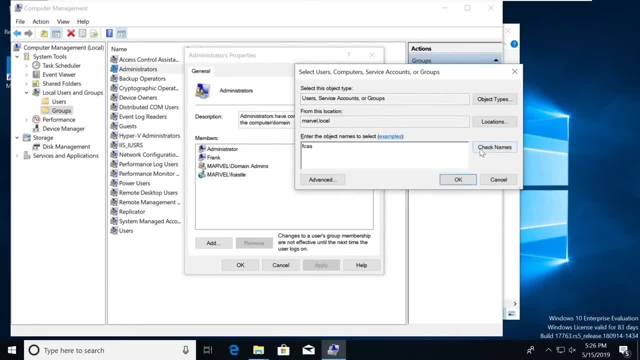 have to do is type in the name of the person. so, F Castle, you can just hit check names and it'll pull it in if it's in the active directory environment, and then you just hit ok, now I've already got Frank in here as a local administrator. 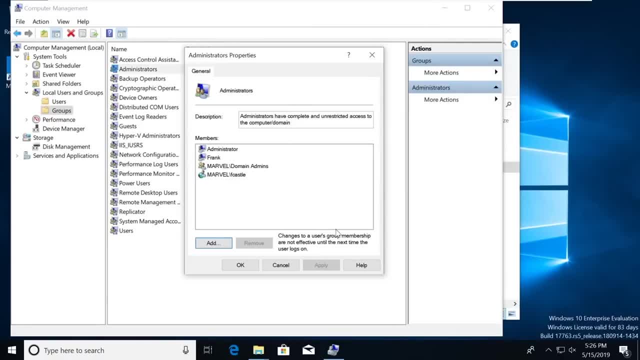 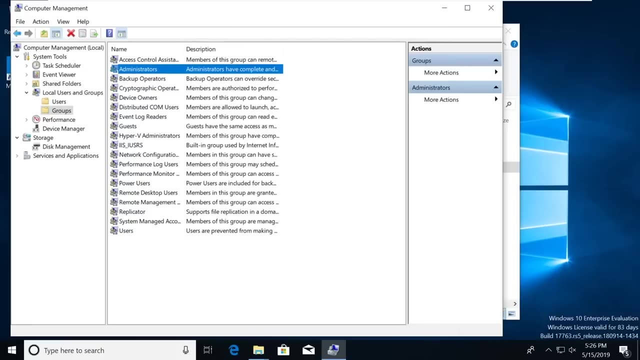 for this computer. thank you solely for the sub. I appreciate that. all right. so we've got Frank in here and we've got him as a local administrator. we've got a scan share that he can access via SMB. so what we're going to do is we're going to go ahead and create a local administrator for this. 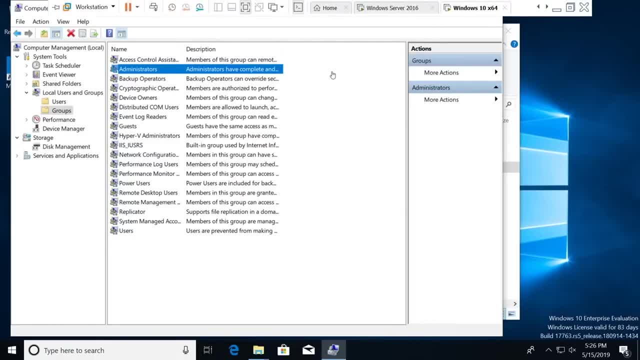 information figure here, right, so we're gonna go ahead and say that I'm gonna permit Alexander Monahan and I'm gonna help him do it. so I give you to an schlimp which you like, let me do it. so let's do that then. then then excuse me, I thank you that you пери редs. 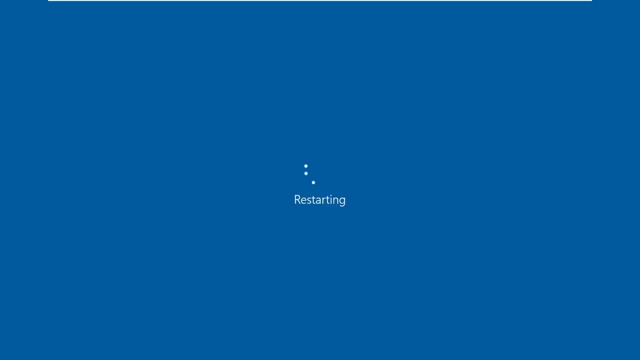 and okay. so somebody asked I'm gonna answer some questions while we wait. so somebody asked if I think sansed cors, jis are worth it, like the audience was saying, if you have the funds to pay for it or for some type of service or stuff like that. so I'm gonna ask that person if they need to pay for it, in case you need in an otherwise or other way, if you already nominated anybody for funding or game over time. so ideally if I can grab on, but then if you have access or any other website, you'd obviously need a excellency or money or the full bonus. 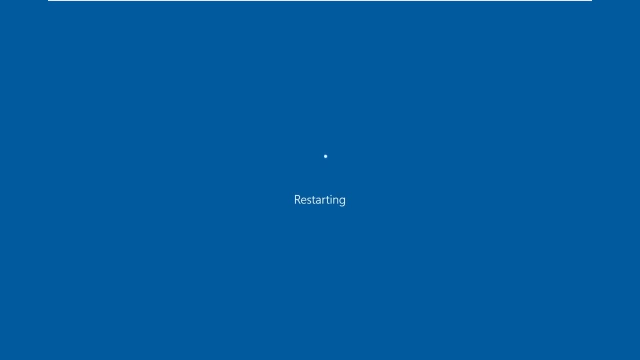 if you have work funds to pay for it, then I think it's a good opportunity to go. They also do have the work study program where you go work for a week and then I believe it's like $1,500 or so to actually take the course. So things to consider, but you can spend your money. 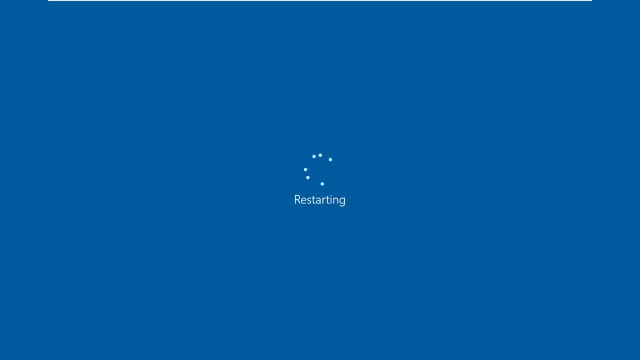 better elsewhere, unless you're working one of those cush jobs that actually do pay for your SANS courses. Now you can see that I'm stuck in the restart loop from hell, so it may be a minute. I rebooted this machine earlier and it took its sweet time, so 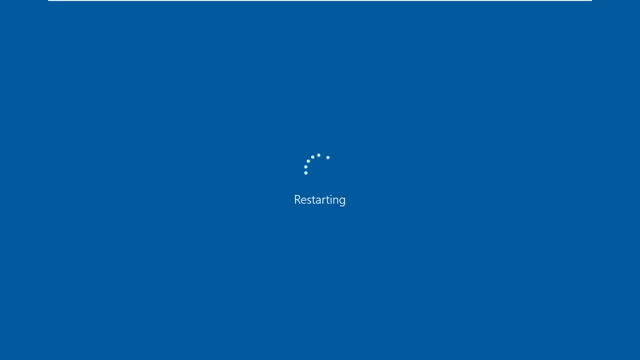 I don't want to force shut it down if I don't have to. Jeff says the military has a free program. While we're doing this, I'm going to bring up the chat so people can see what's going on. I'm going to bring up the chat so people can see what's going. 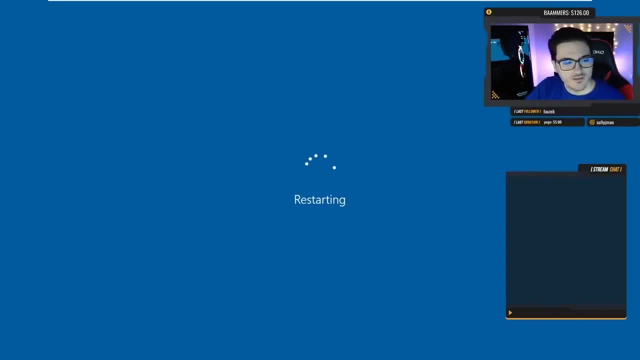 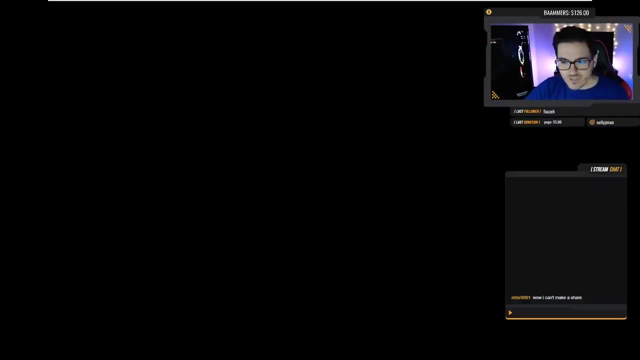 on. I'm going to bring up the chat so people can see what's going on. I'm going to bring up the chat so other people can see if they're watching. You can't make a share. Why is that? Updates. The Bucks play in two minutes. The Bucks are going to lose. 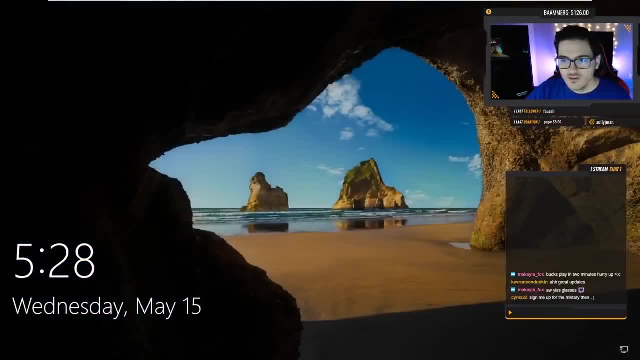 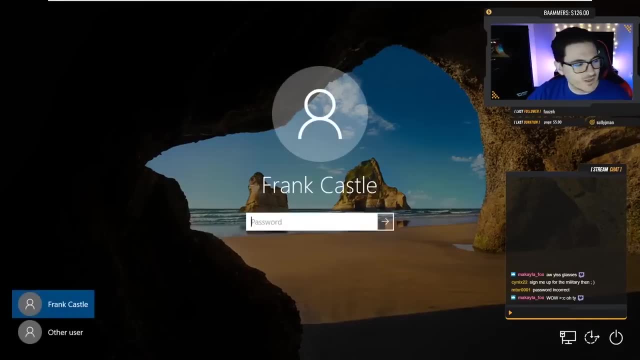 I don't think so. I think the Bucks are going to win the series, if I'm being honest. Password incorrect: You forgot your password. Password incorrect: You forgot your own password. man, Come on All right When you get to the login screen. if you worked ahead of me, this is why you are wrong. 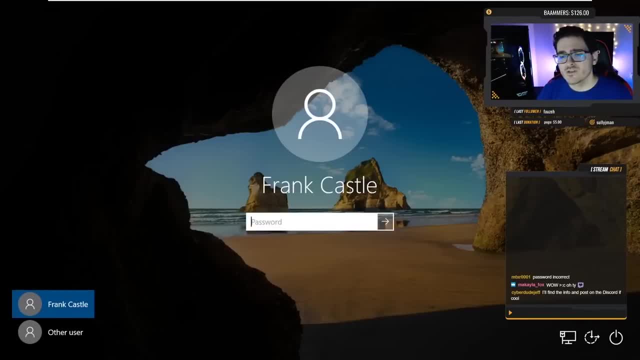 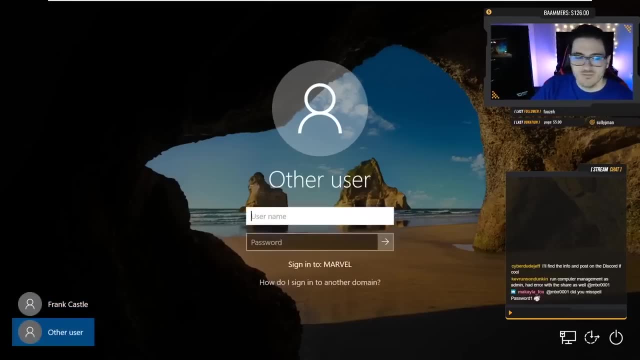 When you get to the login screen, please do not log in as Frank Caslow. We're going to perform two attacks today. Please log in as the administrator, the domain administrator. So Marvel, and we're going to log in as administrator. 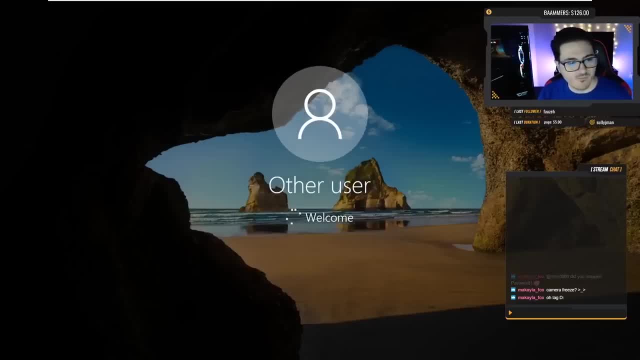 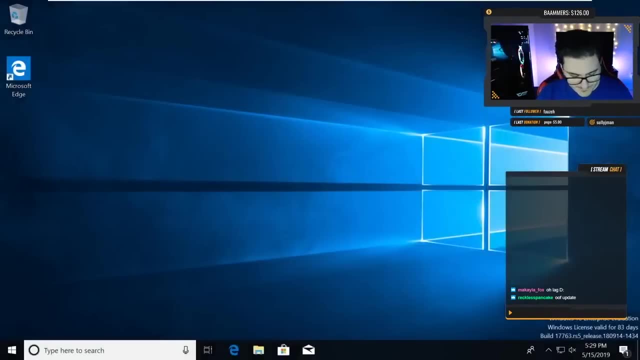 Hopefully you remembered your password from last week. I will give you guys time. I know I also ran into the update as well. So Windows forcing updates on us whenever they feel like Feels bad. right, So we're logged in. Make sure we're logged in. 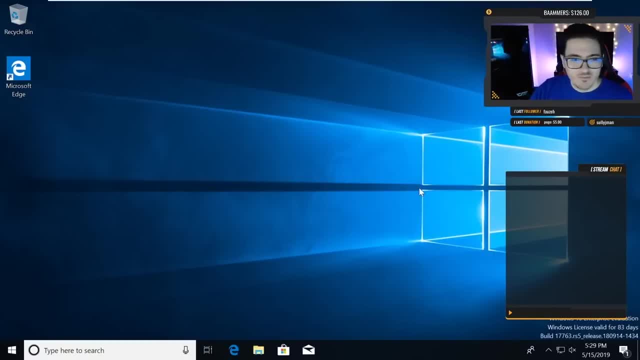 sure when you get logged in, you're logged in as an administrator. I'll give it a couple minutes. if you got a question, I'll. I'll wait for you, some of you, to catch up, and also I'm gonna give some credit to Windows Defender, because Windows. 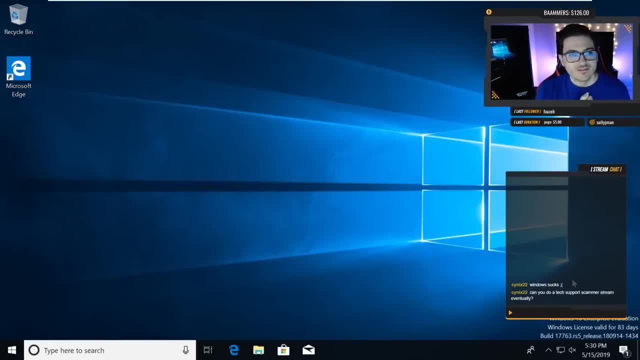 Defender has caught me in the last couple weeks doing exploits that I have never seen it catch me before, so it's gonna be time to start upping my game. so I'm- I'm honestly really impressed by some of this. so we're gonna actually have to turn off Windows Defender for the exploit we're about to run and this: 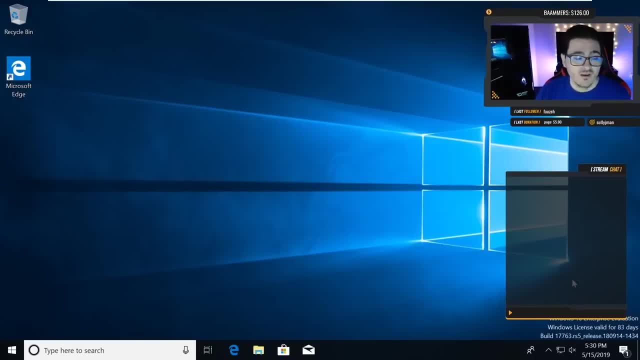 is an exploit that I run all the time in client environments, whether or not they're using defender. most likely not probably some form of AV that's not catching this, but defender is doing a really good job as of late catching catching these exploits. all right, so we are logged in. 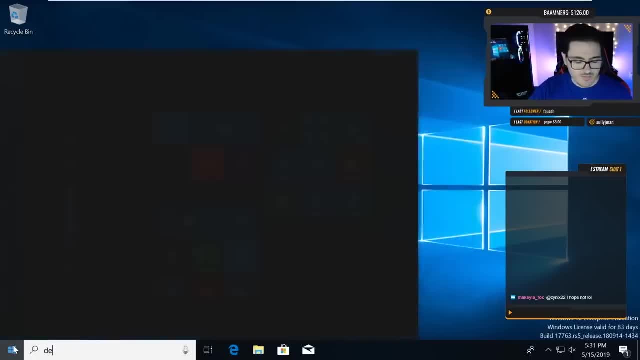 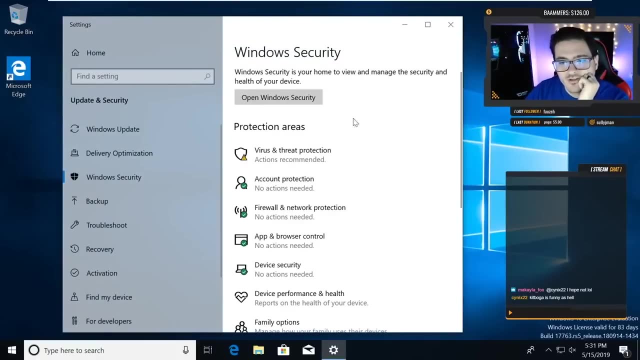 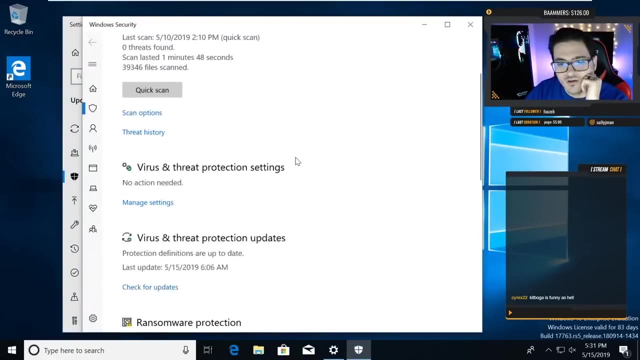 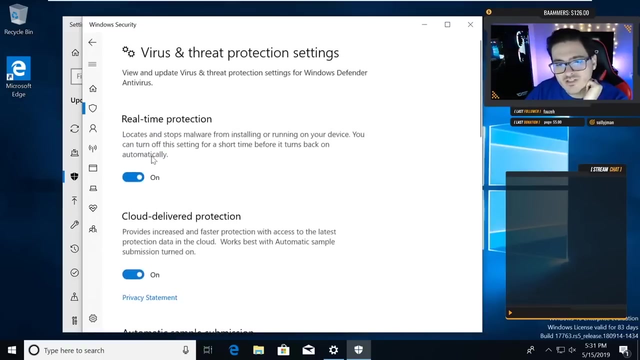 as the administrator, I'm gonna go ahead and just get it going. I'm gonna type in defender, go to Windows Defender settings. we're gonna click on virus and threat protection and I never know how to disable this. there we go, go to manage settings and we're gonna turn off real-time protection. you didn't see that I will. 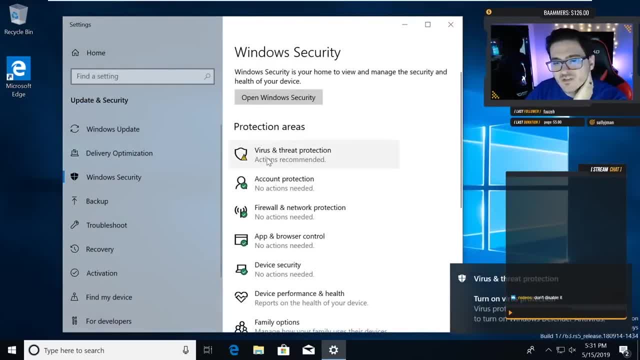 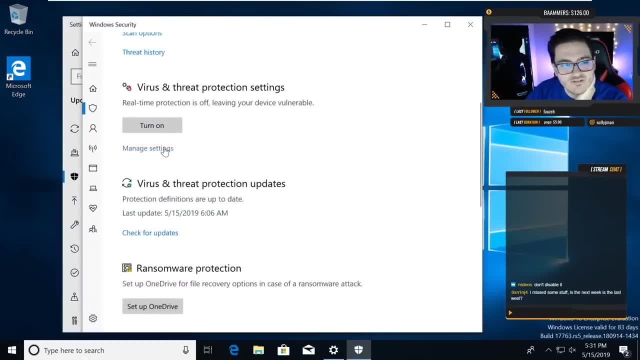 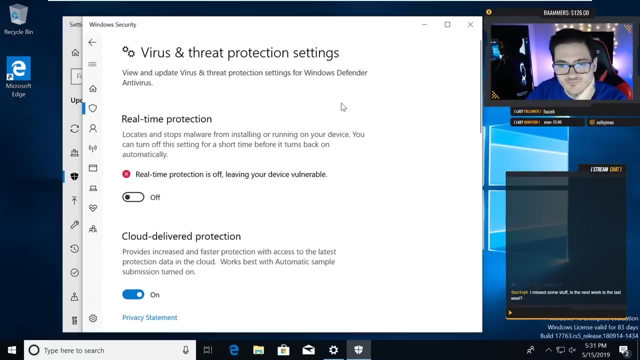 repeat it: go to Windows security, click on virus and threat protection. you're gonna manage your settings and then you're gonna turn it off here in the real-time protection. Niden's the saying: don't disable it. he's warning us for the bad things that are. 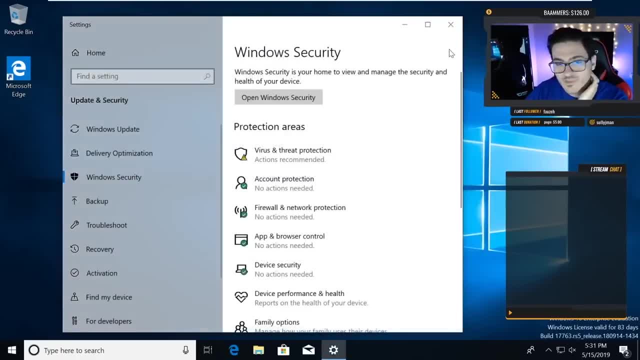 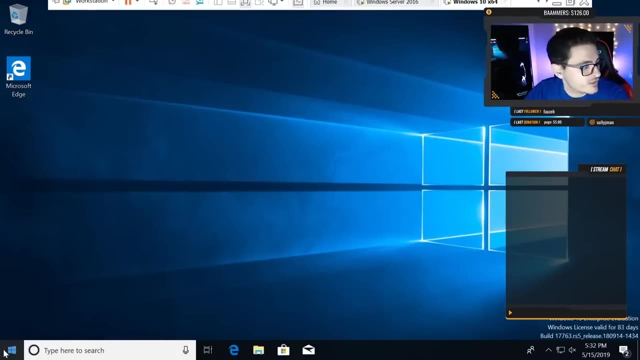 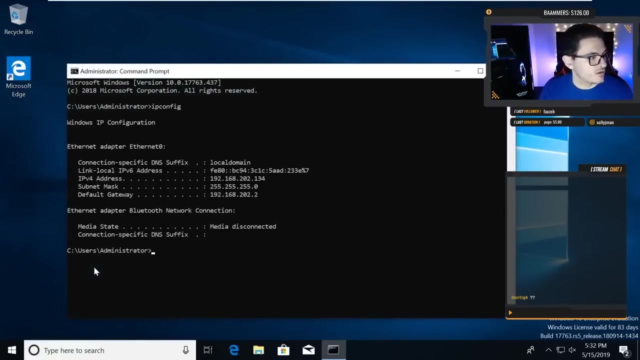 going to come all right. so now we've got that disabled, we can stay logged in. doesn't really matter. let's go ahead and hop over. actually, let's get the IP address of this machine to make sure that we are attacking the right machine. sometimes these things do change. it is one, three, four. earlier it was 138, so that's good to. 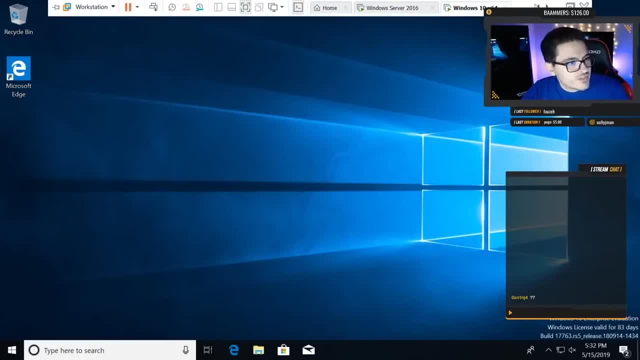 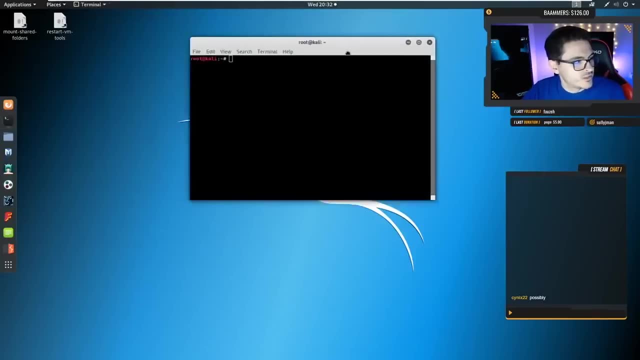 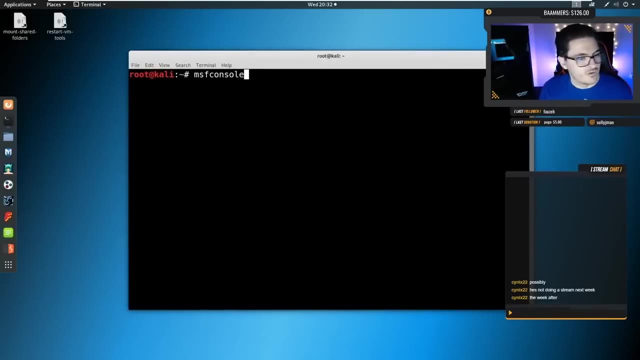 know. okay, so with your IP address in hand, go into your terminal. we're gonna be living in Metasploit. I'm doing a stream next week. guys, thank you for watching this video. hope you liked it. I appreciate it. Subscribe, like, share and hit that like button. see you next time. 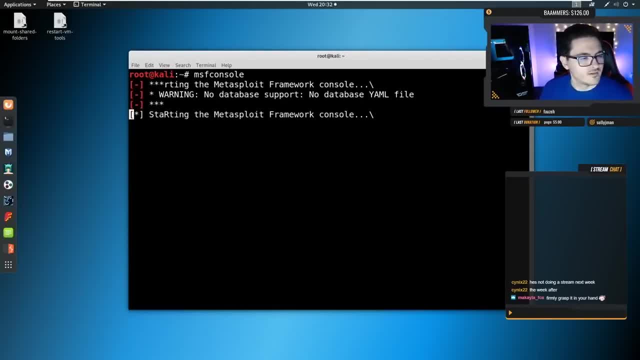 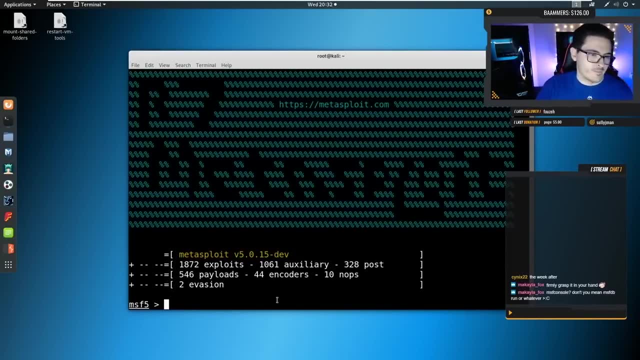 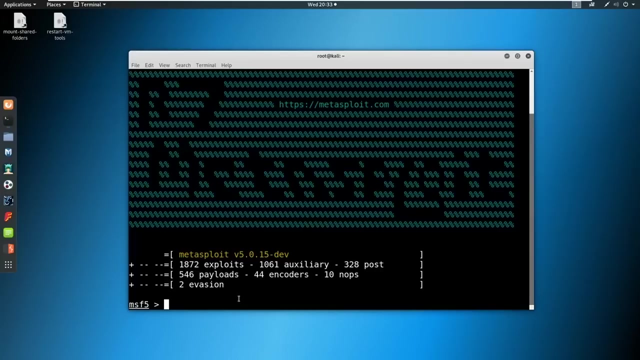 week. Don't spread lies. Gray's over here spreading fake news, All right. So we should be at this MSF5 screen- I'm going to take my face away so you guys can see everything- And we're going to be using a tool called PSExec. So we're going to say: use. 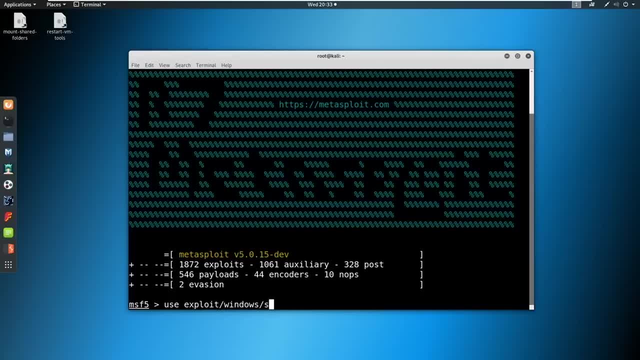 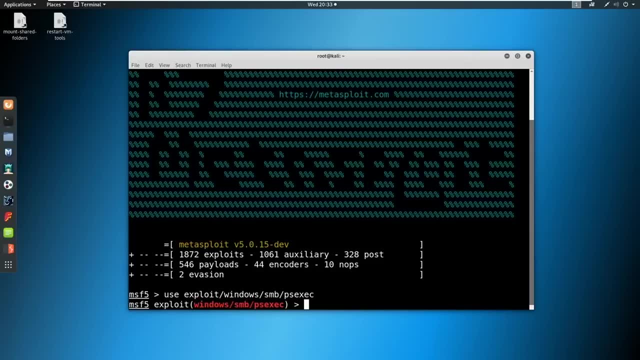 exploit Windows SMB, PSExec, Just like this. Now, what this does is, if we are able to connect to a shared folder as an administrator or with execute privileges, we can upload malware and gain a reverse shell. This is important, So there are two tools that we're going to actually use. 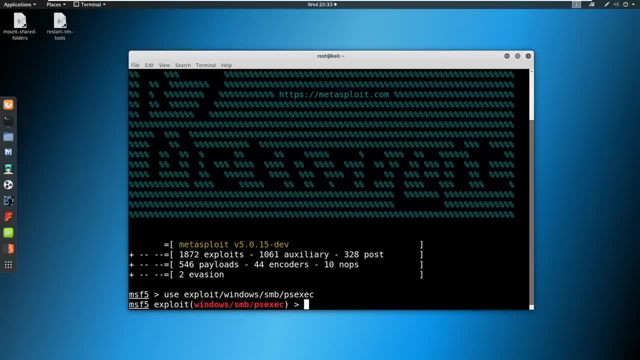 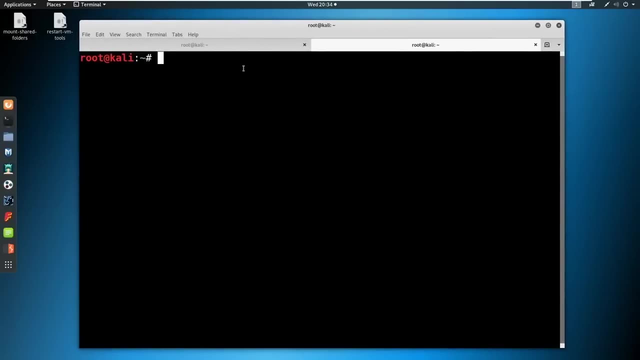 Actually, let's back off. Let's back off. This would not be my first step. Let's back off just a little bit. So actually let's do this: Type apt install. And then I want you to type crack map exec, just like this: 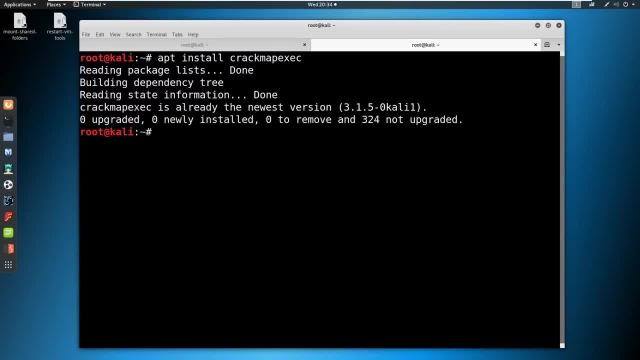 And hit enter. Now I've already got it installed, but go ahead and install it, I'll give you another second. You said you heard I was giving away a ThinkPad. You know, nobody has sponsored my stream, So if you call Lenovo up and you get them, 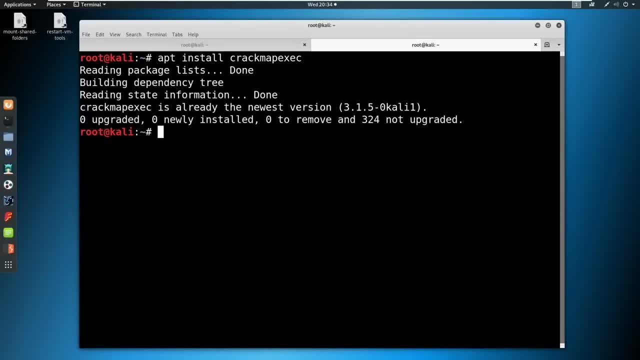 to sponsor my stream. I will give away that ThinkPad. All right, You can be my marketing outreach, Jeff. that can be your job, since you're going to be doing nothing else in Amsterdam. All right, Let's say that we've got crack map exec installed. 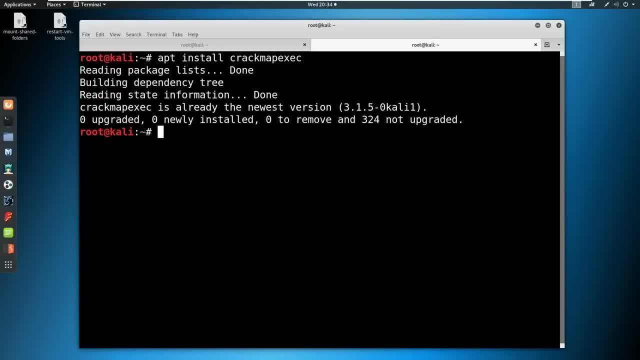 So I'm going to give you a proof of concept. here We could use the credentials we already have. We're pretty much only going to log into one machine, which would be our machine. So I'm going to give you an example A little bit different. 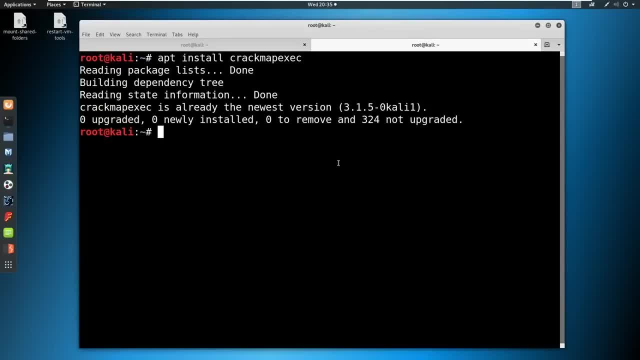 So crack map exec what it does is it does a pass the hash or pass the SMB account or whatever account you've got, depending on what's built in. I don't know. I only use it for SMB. I think it has more than that. 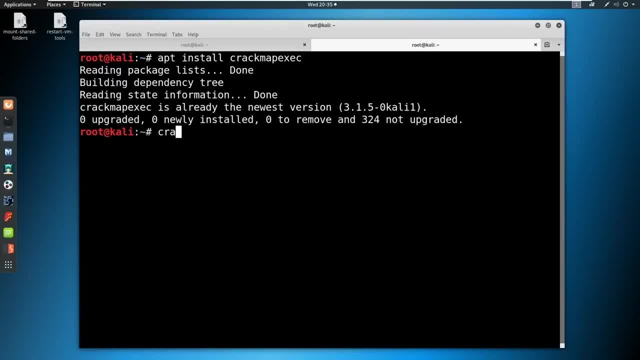 So what we're going to do is we're going to say crack, map, exec, And you'll understand more once I type in the syntax here. We're going to say SMB And then we're going to type in the targets. So for me, I'm actually going to type 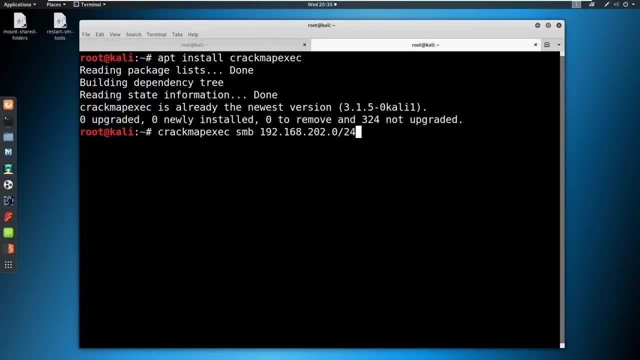 You could type an IP, one IP address. I'm going to type in a .0 slash 24.. And what it's going to do is it's going to sweep the entire network with the credentials, looking for SMB logins, And it's going to come back and say, hey, I found a login or hey, I didn't. 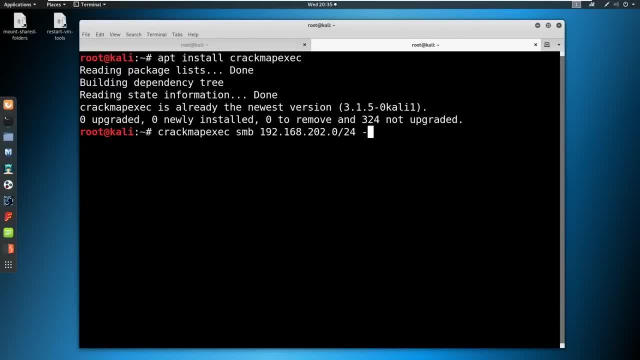 This is a tool by Bytebleeder. It is an amazing tool. So we're going to just say username, dash U for username, administrator, Dash P for password, And make sure you put quotations around it. Whatever your domain admin password was, please remember that. 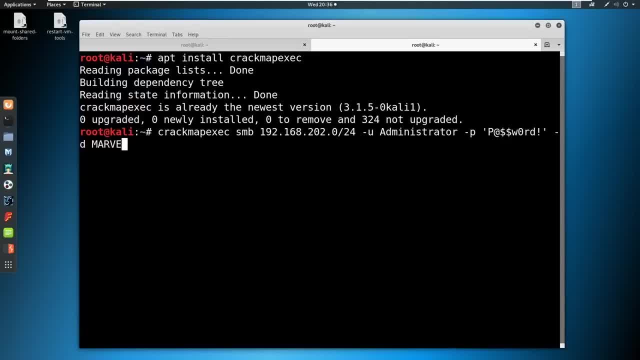 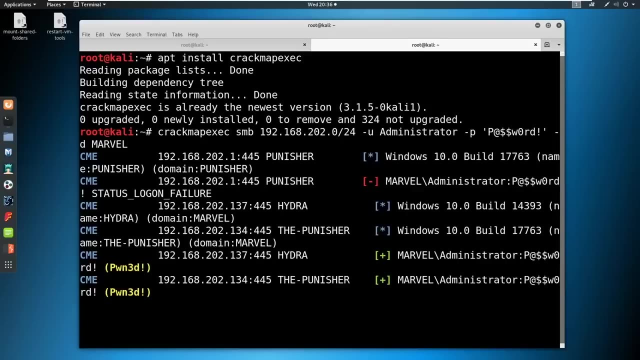 And then a dash D for domain. Our domain is Marvel, And then we're just going to hit enter on this And that's going to go through all the IPs And try to log in And you can see that it actually pwned multiple machines. 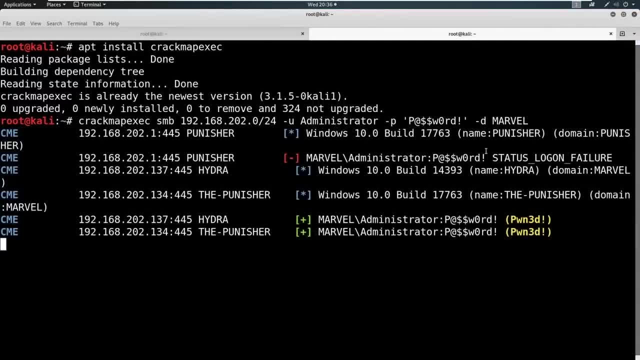 So when you're in an environment and you've stolen creds or cracked creds, what you can do is you can take the creds and you can pass them around and see where you have access to, from an SMB perspective, Every single place where it says that I've got a login. I'm going to go and try to get a PSExec shell. 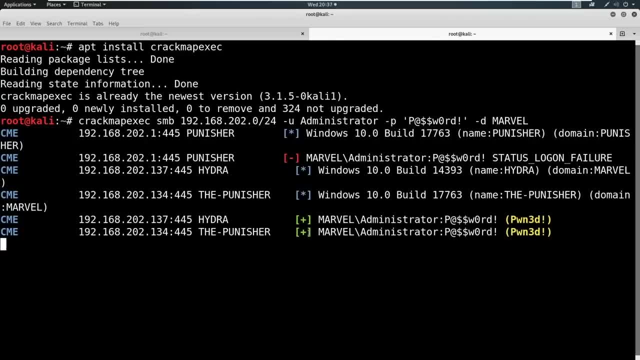 and use that to see what information is on the computer, And we'll talk about that in a little bit. I'm going to talk about that here in a minute, what we can do once we're on a computer. Now you see, the domain administrator has access to all the machines that we have. 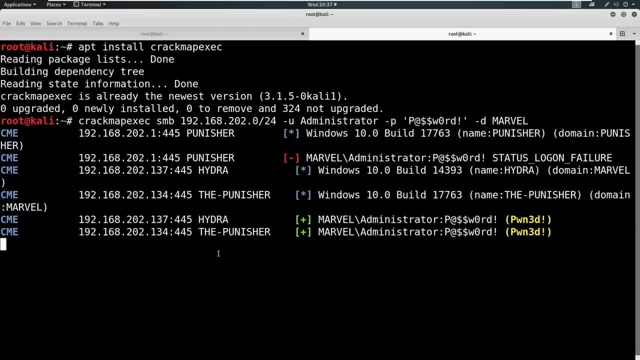 one being the domain controller, the other one being the punisher. The punisher does not have access to the domain controller, which is why I showed you the domain administrator account, so that you can see multiple logins at once. So just know that this tool is one of the best tools you can have on an assessment when you crack credentials. 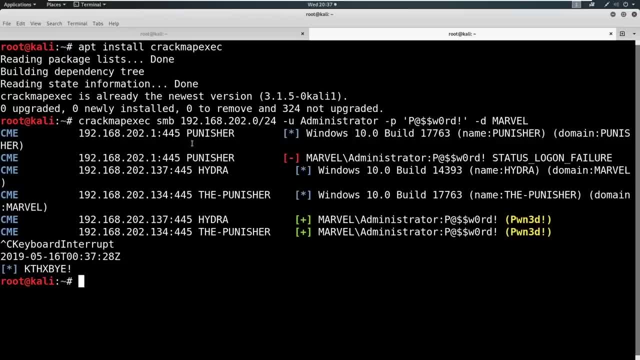 And it also works with hashes, Which I'll show you later. I didn't get the pass the hash to work. I'm going to show you the techniques, but I wasn't able to actually get it working. But you'll at least get to see how to accomplish it. 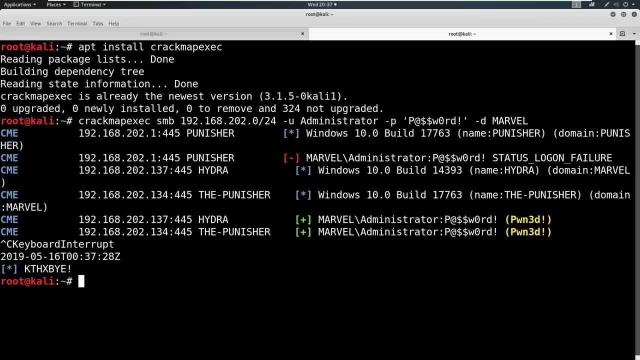 One second, I've got a sneeze, All right. so now we passed it around. we figured, OK, we we're going to try to log in. We'll just pretend that instead of administrator, this was Frank Castle. Oh, thank you, Matt. 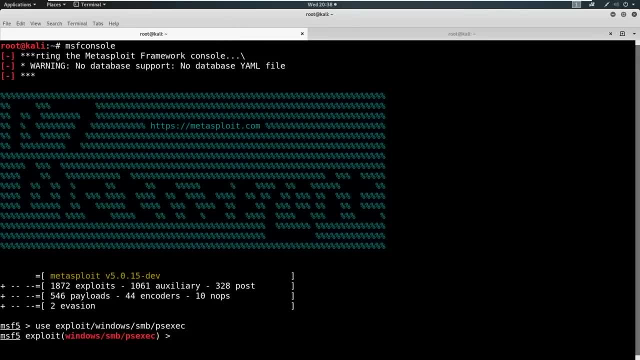 And we're going to come back to our screen over here And we've got PS exec up. So somebody asked we're logging in as domain admin to remove Windows Defender. that is not the case. There's another reason: we're logging in for domain admin and I have not gotten there yet. 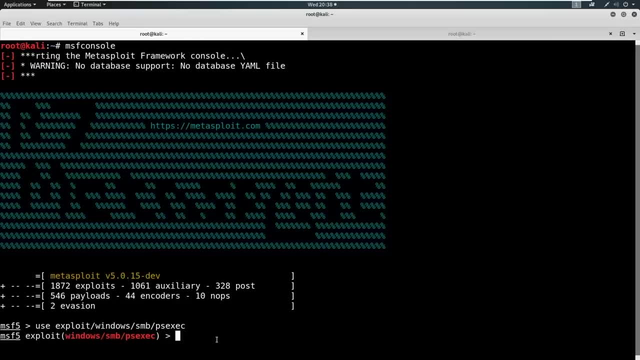 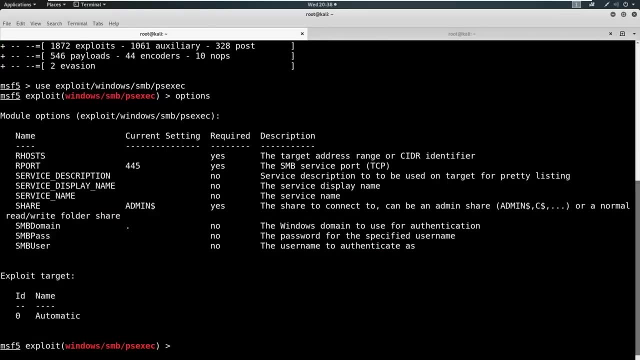 So just just bear with me, The local admin of Frank Castle would be able to remove the Windows Defender as well. OK, So let's type in options And let's set our our host. so my our host was the Punisher machine, which sits at 192.168.202.134.. 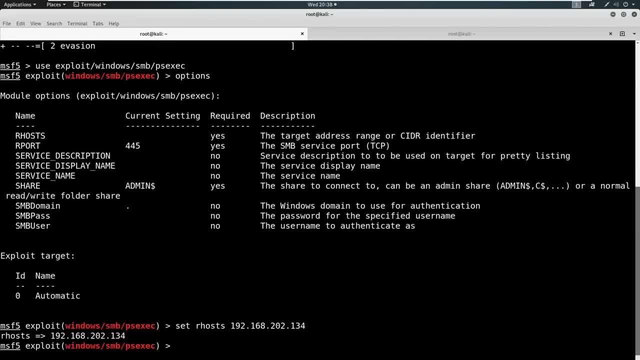 The share of admin is fine, because we need to be able to connect to a, a admin account, to be able to exploit this anyway. And now we need to set our admin. OK, So let's type in options. We need to set a few things. 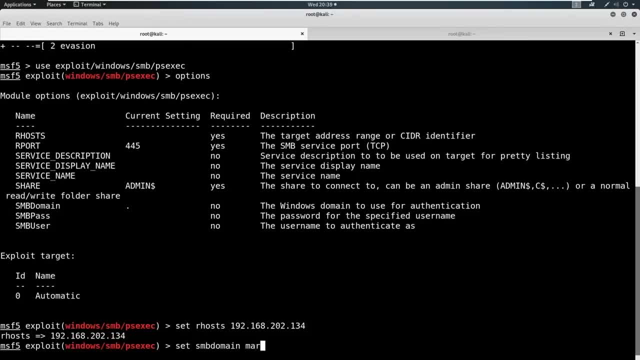 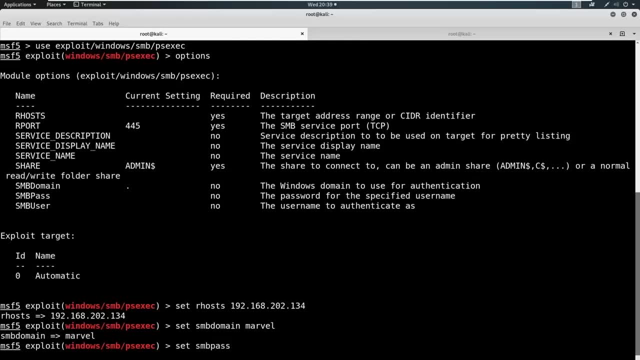 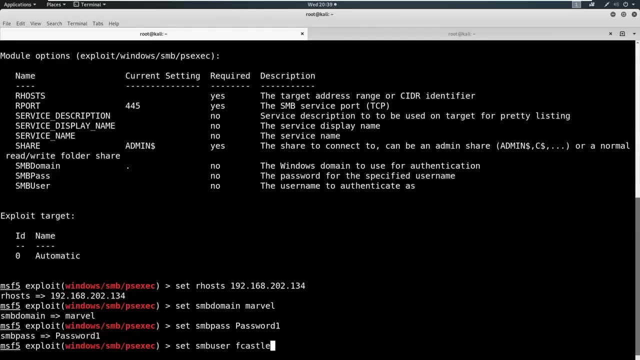 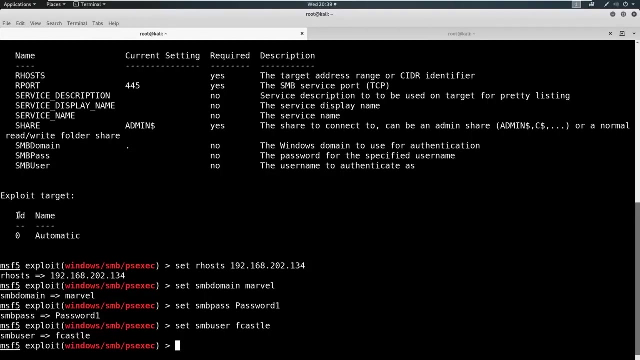 We need to say set SMB domain, It's going to be Marvel. Set SMB pass And we're going to say password one Set SMB user: F Castle, OK, And then down here it says exploit target and it gives us automatic. 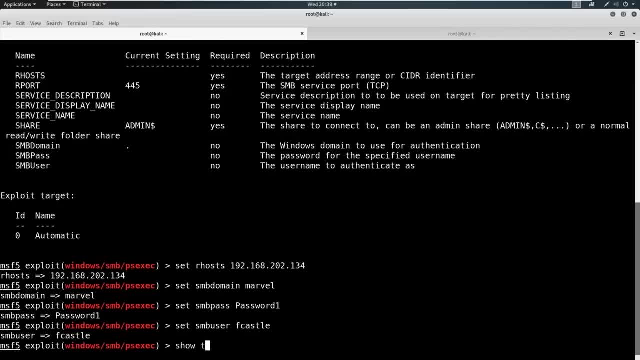 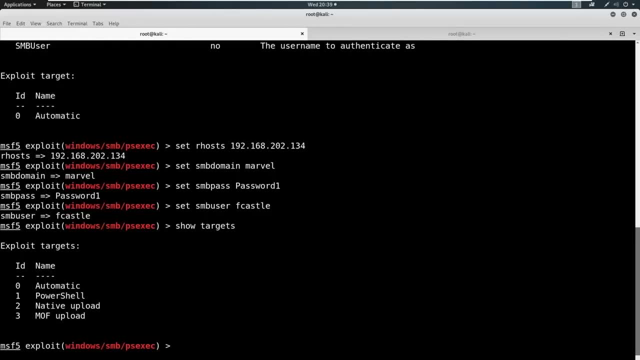 But that just tells us that there's some other targets. So I like to say: show targets and see what possible target options we have. So it's got automatic. It's got PowerShell native upload and MOF upload. I don't have a lot of success with the PowerShell version. 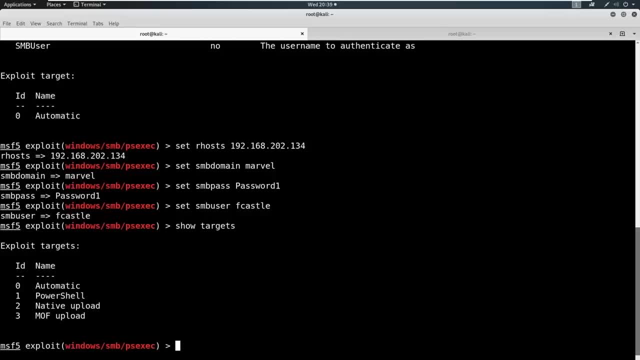 I actually have the most success with the native upload. But when I'm doing this on an assessment, I will run through every single target type. But for tonight we're going to go ahead and just set the target to. So we'll say: set target to. 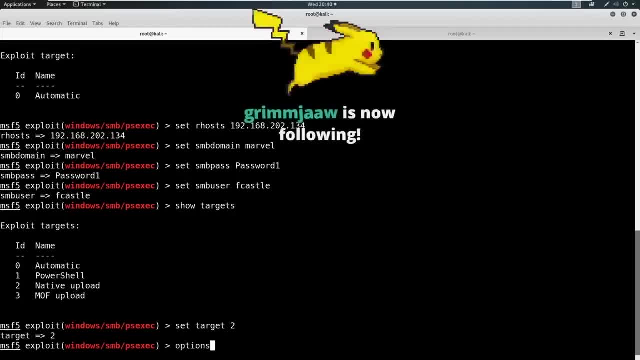 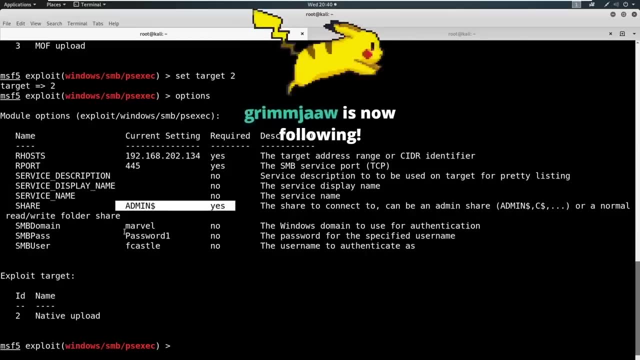 OK, And then we'll say options again to make sure that we have done everything we needed to do. We've hit our required here, required here, and then we filled out everything we need to fill out here. OK, So let's go ahead and just say run. 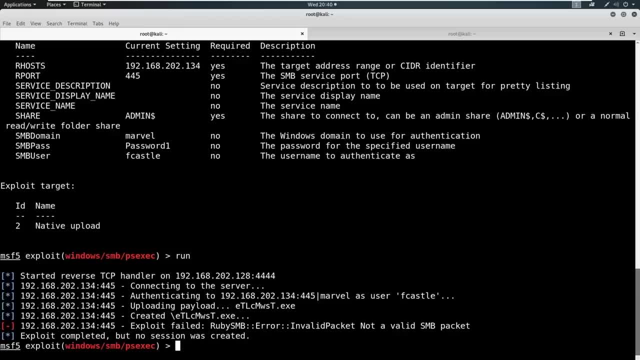 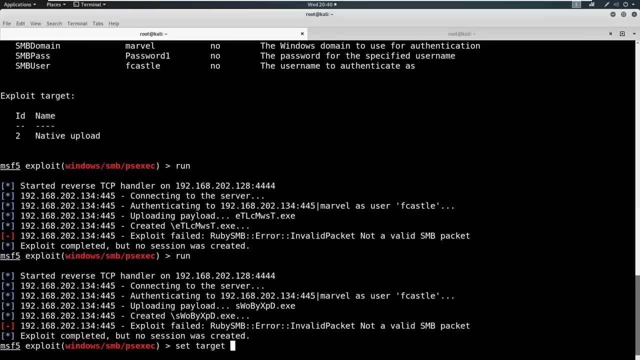 And it looks like we connected, uploaded. It didn't work. We'll try running one more time. OK, Let's try setting the target Something else, See if it runs And that works. So here I go talking about PowerShell never working. 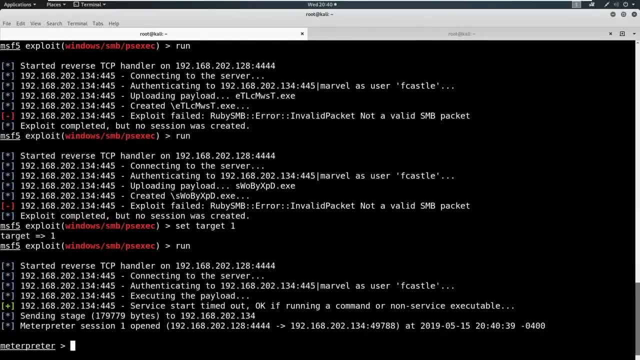 I bash PowerShell And then PowerShell comes through in the clutch. This is what I mean by trying all your different targets. I would stray away from using automatic. You can try it- But I like to go through the targets one by one, if I can. 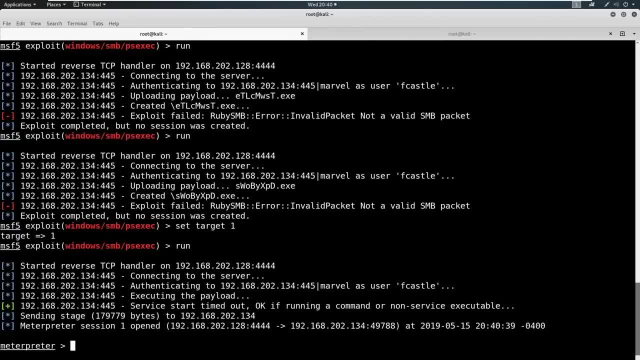 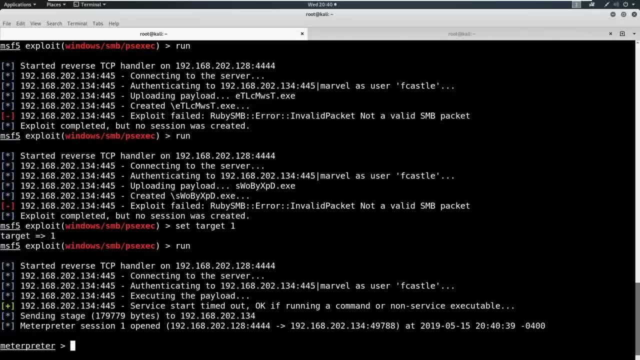 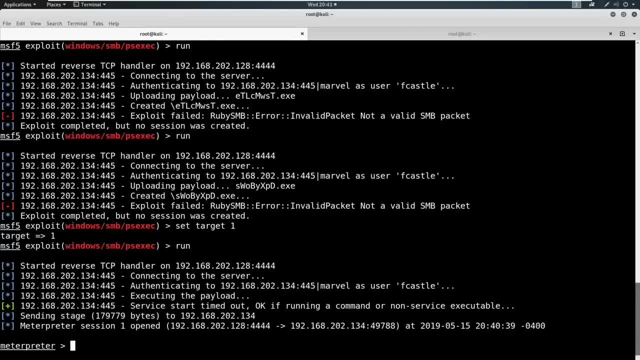 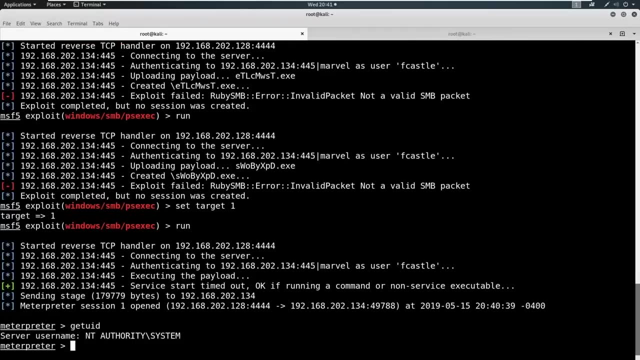 I don't know what it's picking when it's picking the automatic. So now we are in a meterpreter session. You can see it says meterpreter session one opened. We have a shell on this machine. We can say: get UID and see who we are. 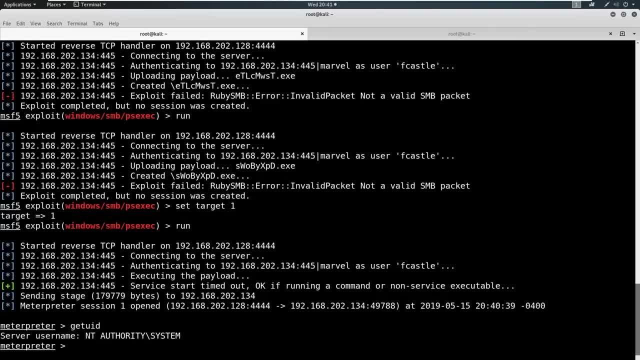 We actually have a shell system, So typically I was looking for this to execute as a render as Frank Castle, And some of the times I run it it does come through for Frank Castle. Sometimes I run it it comes through as system, So not sure why that is. We can type in sysinfo. 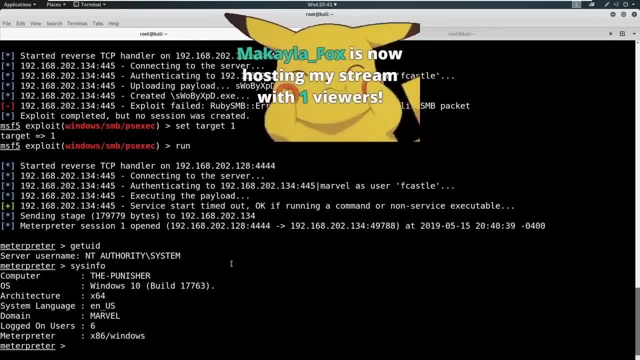 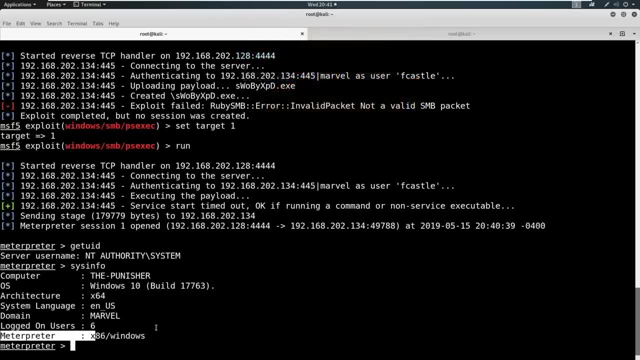 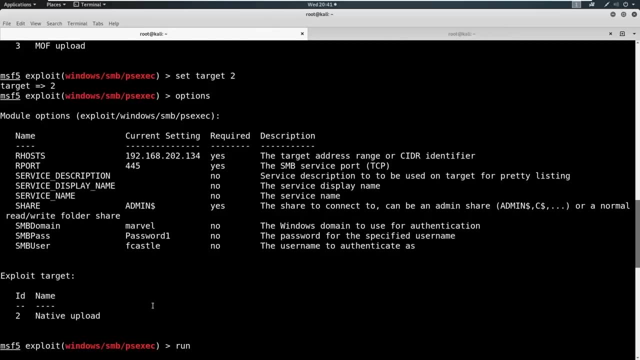 and see what kind of info we have here. Hey, thanks, Michaela. Okay, so we actually got an x86 meterpreter session and we've got an x64 architecture. That's not the best situation to be in, So let's- actually let's- background this. 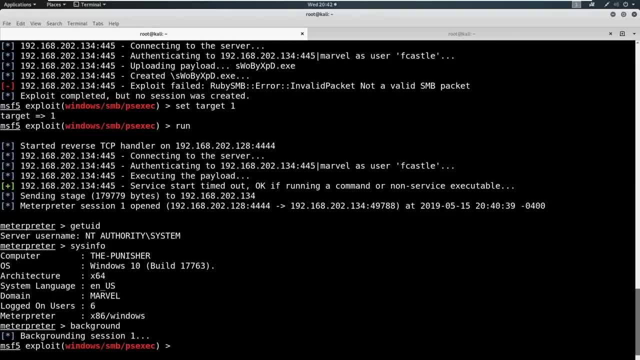 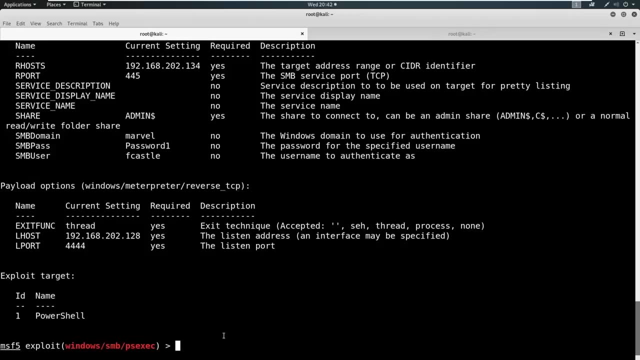 Type in background And it's going to background the session. Let's see if we can't upload another, a different payload. So let's see if we can say: let's look at options. It might not show as okay. it does show as Windows meterpreter versus TCP. Let's see if we can get it into a 64-bit. 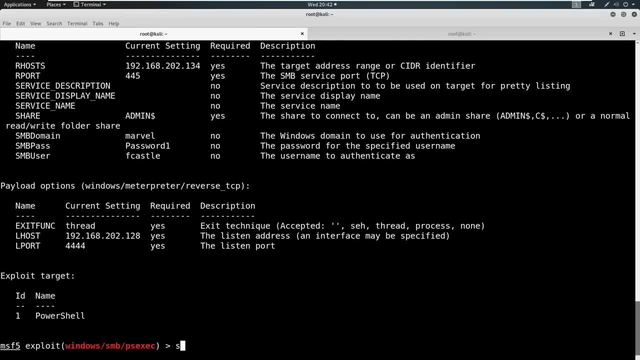 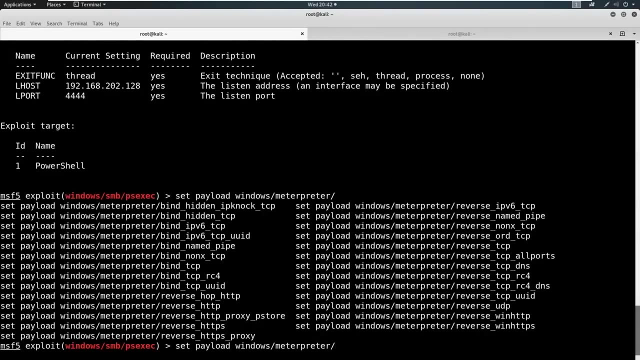 payload And we might not be able to. So we could just say: set payload Windows interpreter double tab And there's actually not going to be a 64-bit payload, So these are all going to run in as 32-bit And people are getting ahead of me. Yes, yes, yes. So we're here. 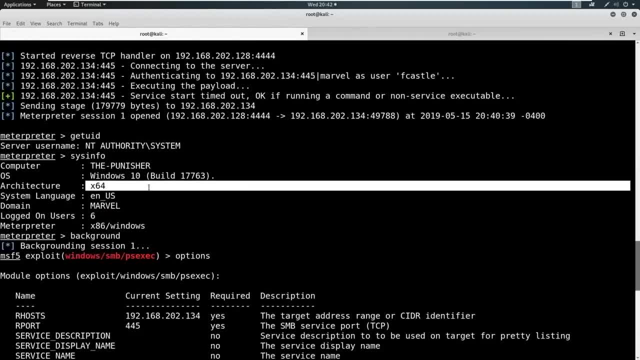 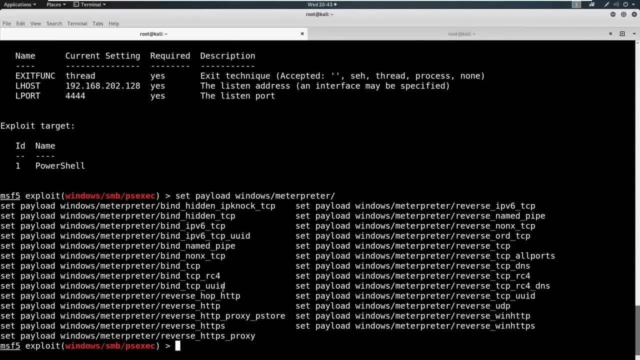 in a 32-bit situation, right, And it's always important to know what architecture you're on, what meterpreter shell you have. Can you improve that shell to get where you need to be? So we cannot here. We can't get any better. So what we're going to have to do is we're going to go. 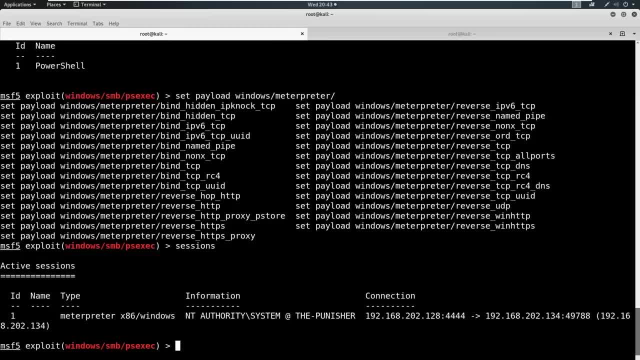 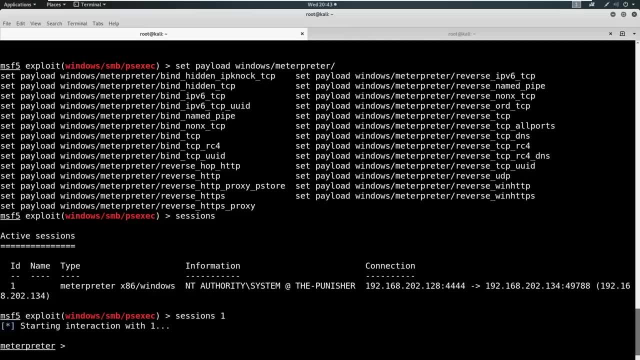 and say sessions. Okay, we've got our session here. We can just go back into session one to say sessions one, We're back where we need to be. Okay, Now Ruri is getting a little ahead of us and saying that we can migrate into a process. So if we type in PS, 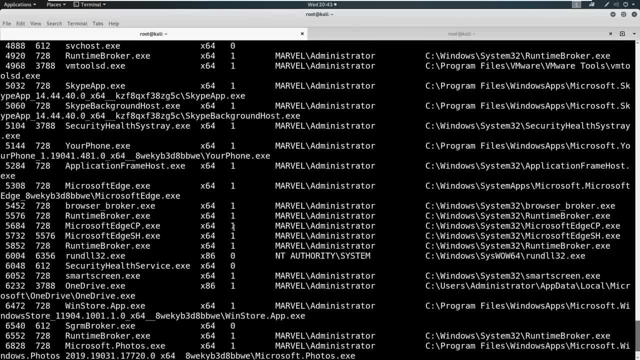 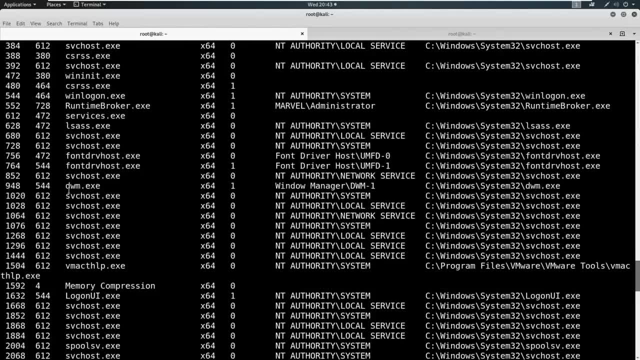 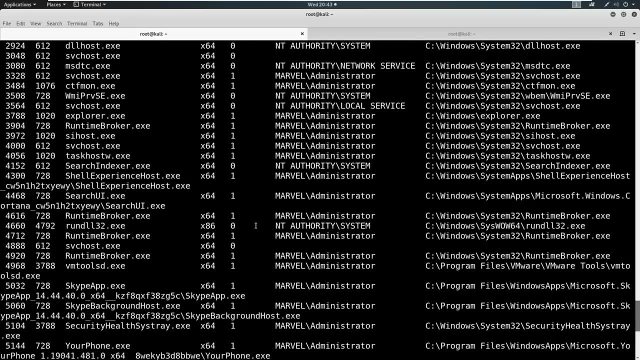 and you look through these processes here you can see all the processes running. You can see the PID and the parent PID. We have to be very, very, very careful of what we pick here, Because if we pick the wrong process- and sometimes it's a guessing game- 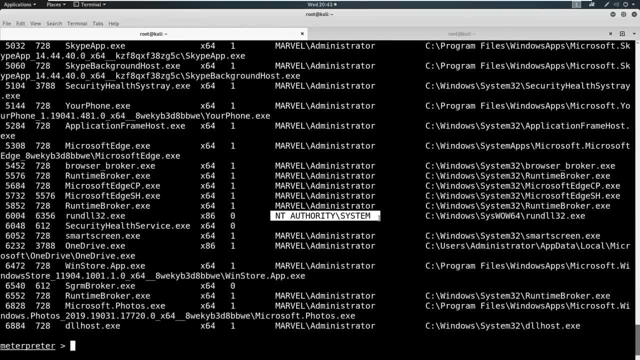 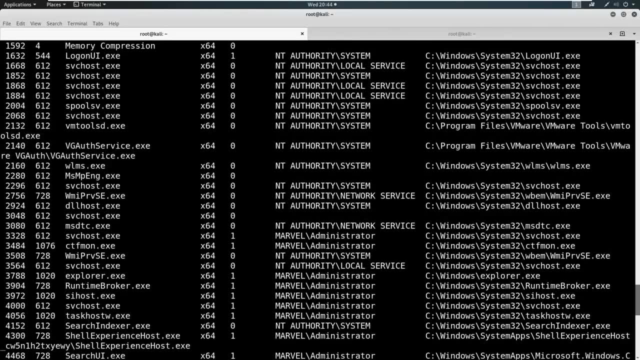 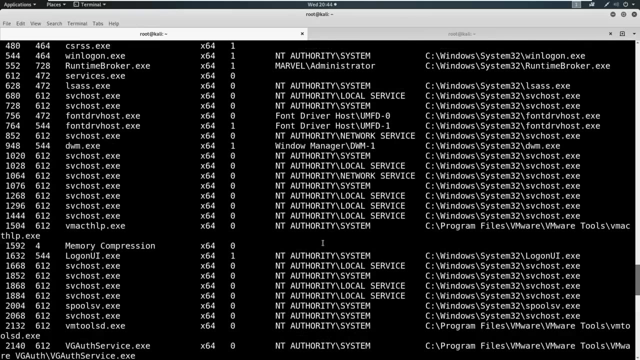 you want to pick something that's running as system already And you want to pick something that's running as x64. And sometimes it bombs the whole thing. So Ruri is saying service host every single time. But I'm not going to mess with it today, I'm going to leave it alone because I've got other lessons. 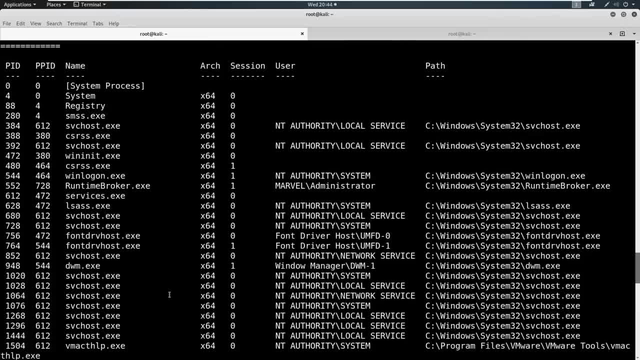 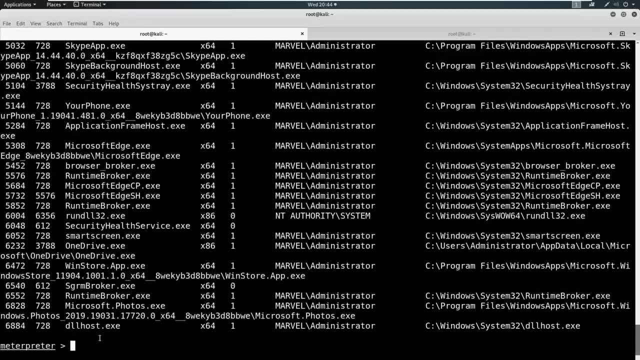 for you guys. But if you're feeling adventurous, you could pick one of these. say example 1076.. You could say migrate 1076.. Hit enter and try to go into it. You may lose your session and have to reboot your machine. 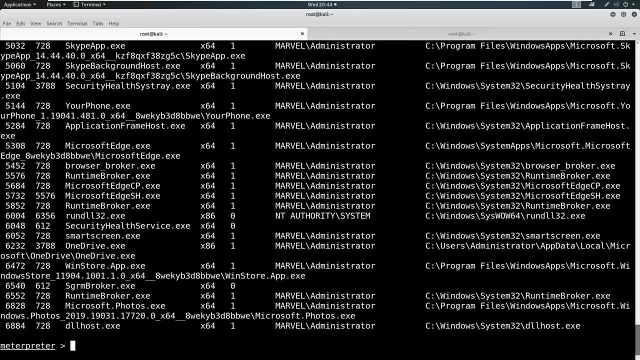 So for purposes tonight, we're just going to go ahead and skip doing that. I don't want to break the machine, have to reboot and have to go through the process again, But it is important to know what process you can, or at least need to switch into. It's important to know your architecture. 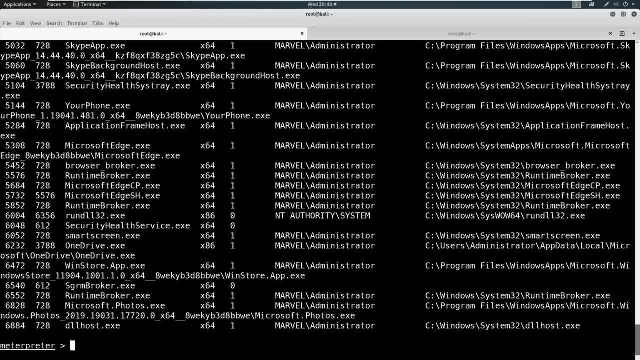 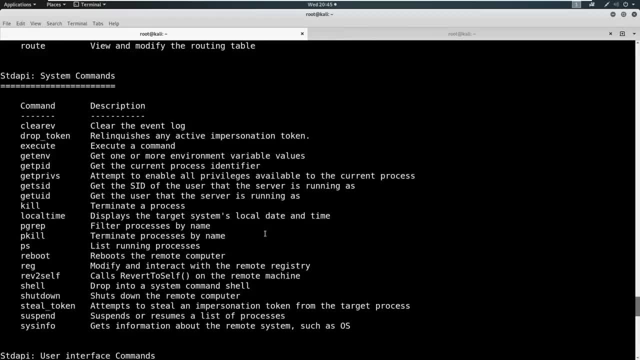 as well. No balls? Yeah, I've got no balls, All right, so let's type help. Let's see what all the fun things we can do with a meterpreter session. There's quite a bit right. So you've got your core commands here. 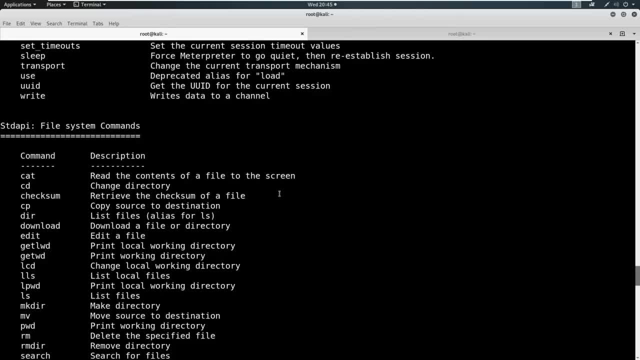 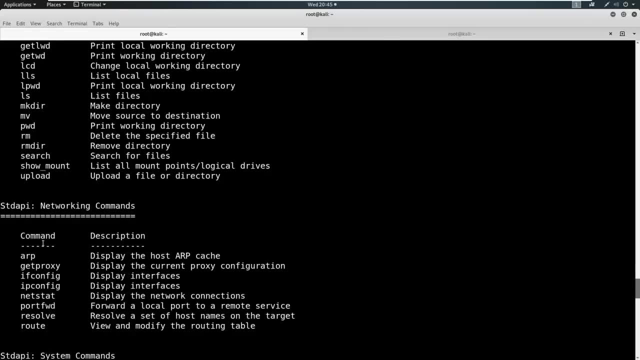 You've got file commands. We can actually download a file from the computer. We can upload a file to the computer. We can navigate around, make directories, etc. We've got networking commands. We've got the fun ones. We've got ARP. We've got route. 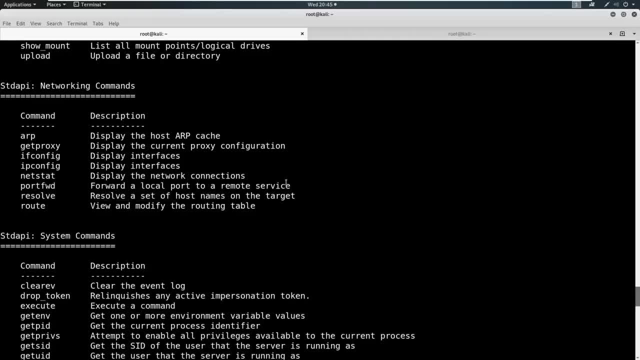 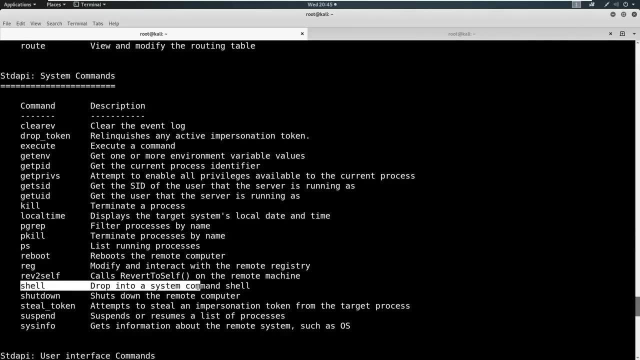 We could do port forwarding, which we're going to talk about in a later video on how to pivot and use port forward. We could see the IP addresses if we need to. There's system commands, kind of what we were just doing. PS, we can reboot it. We can do a shell, which I'll show. 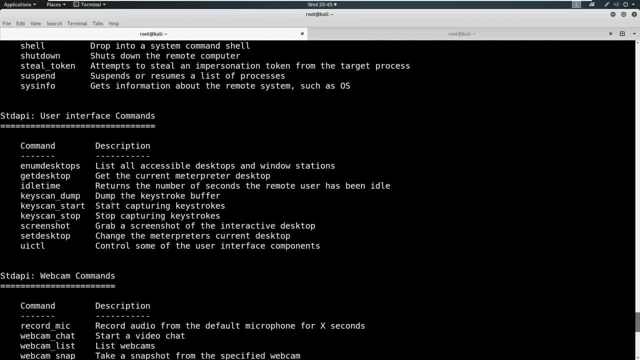 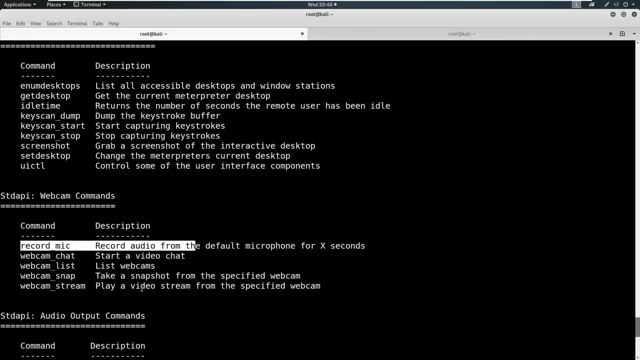 you here in a second. We can do key scanning. We can basically do key logging. We can take a screenshot, We can look at the webcam, We can record the microphone, We can take a picture of the webcam, We can watch the video stream from the webcam. So when you have those little webcam covers, 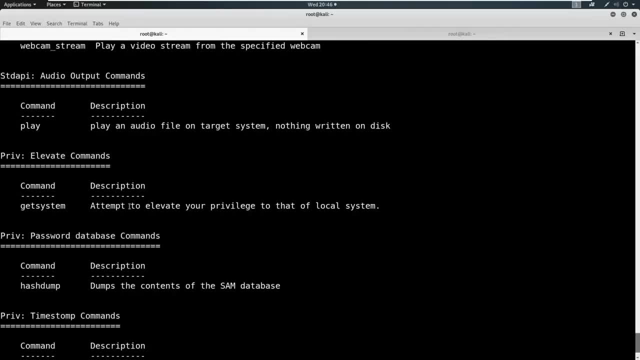 this is a big reason why that you have those webcam covers. We've got elevate commands here. Get system: This is one of the first things that I try if I have a low session And the get system actually works on this one, If you're brought into a session as the administrator or not. 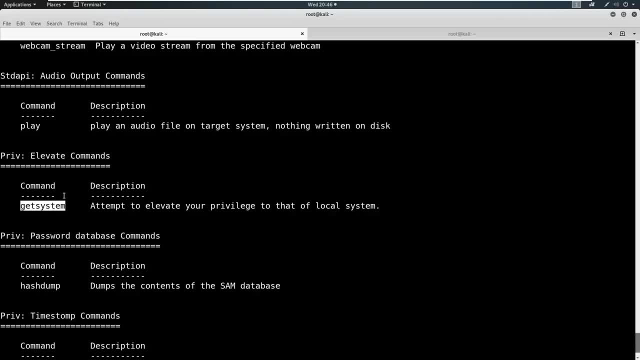 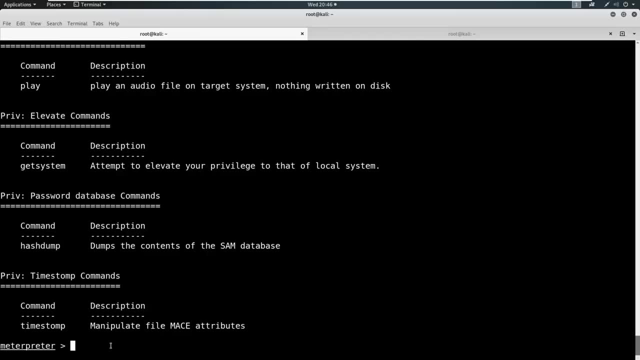 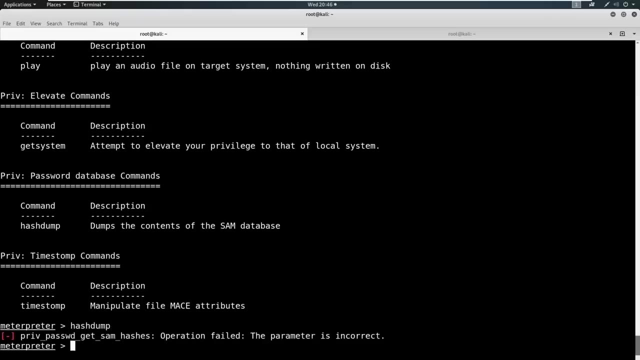 not system. if you just type in get system and hit enter, you will actually get the system. Now, hash dump is one of the most important commands that you need to know. It is not going to work for us in this situation. I can show you. As Ruri said, I have no balls, but hash dump is. 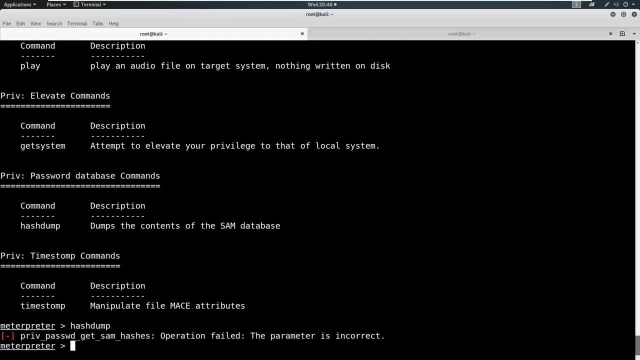 not going to work in this situation because I have a 32-bit architecture, meterpreter, shell and we are on a 64-bit machine. So until I migrate that session over then none of these things are really going to work that well. So I'm going to show you everything conceptually. 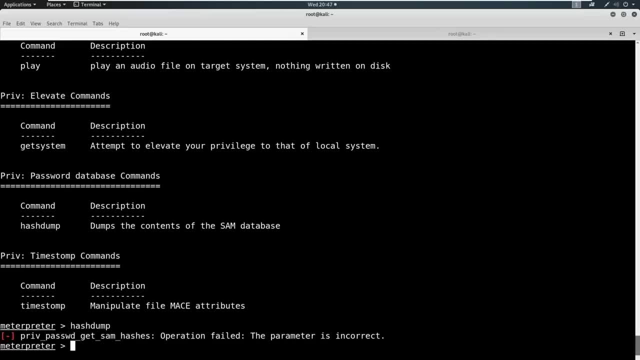 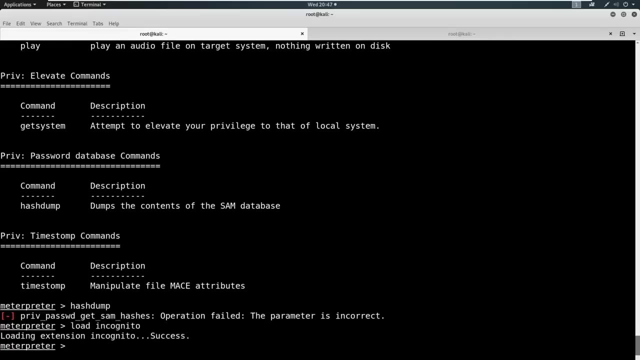 and we're going to go ahead and just kind of look around. So one of the first things that I look for, and what I try to do right away, is I load up a tool called Incognito. Now we're about to do. all you have to do is type, load incognito and if you want to see the incognito, 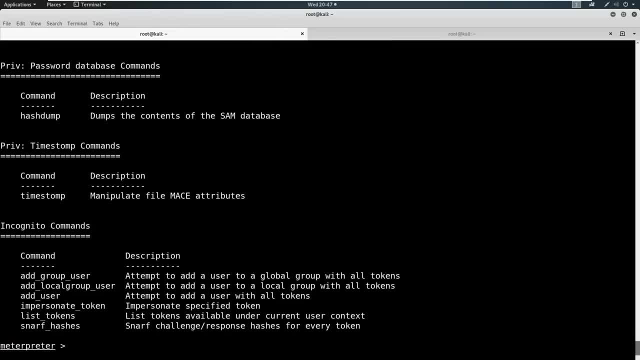 commands you just type help. it brings it down at the bottom, the last loaded module, uh will, will show you exactly all the commands that it has for it. so what we're about to do is called token impersonation, and so let's talk about token impersonation. so you have these things called. 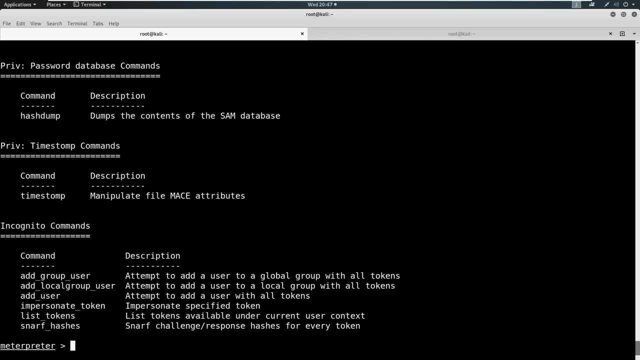 tokens and basically they're just a temporary key, right, um, and it allows you to get in and out of systems and networks without having to do to use your credentials. so what we can do is we can replay those tokens and try to gain access to an account. so there are going to be two types of 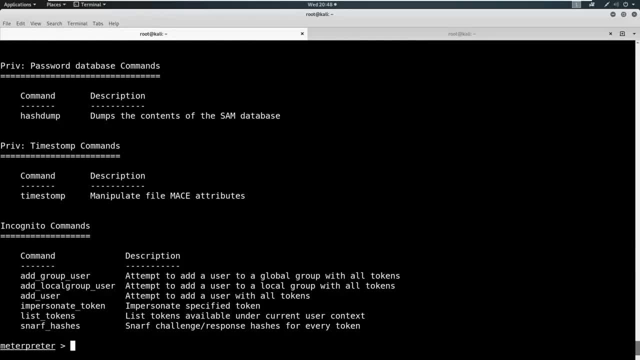 tokens that we're going to see. we're going to see delegate tokens and impersonate tokens. uh, the delegate tokens are going to be the ones that are going to be the ones that are going to be the ones that are for the type of logins that you actually physically log in the machine, like we did with. 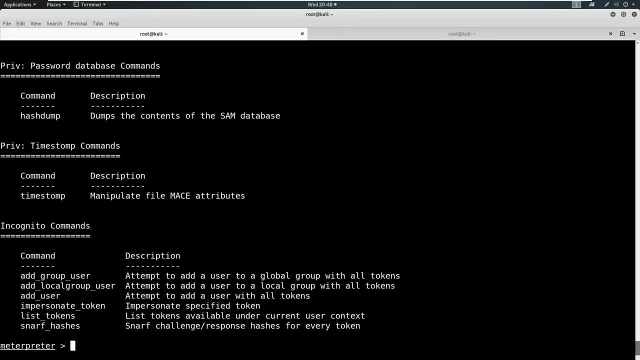 the administrator account or if you do like rdp or something like that. the impersonate tokens are when you're like using a network drive or you've got scripts running or something like that. so it's basically hands-on interacting versus not interacting. so what we can do here is we can say we want to list the token. 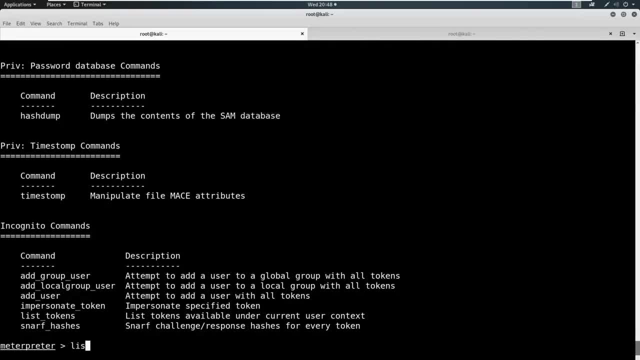 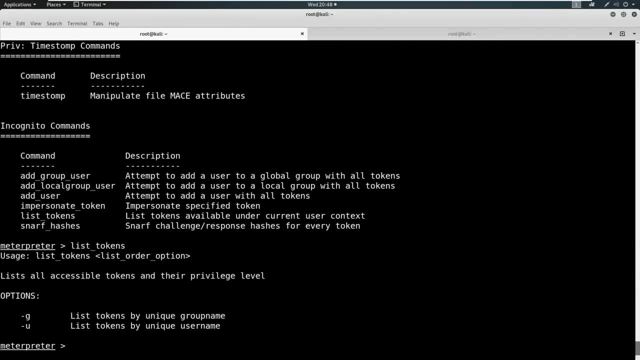 tokens. so we'll do list tokens and then it'll want an option here. if you just hit enter it'll ask for an option. we can either do by group name or by username. i like to do by group or by user. i'm sorry, because by group will throw in quite a bit of information for us. so let's look at user. 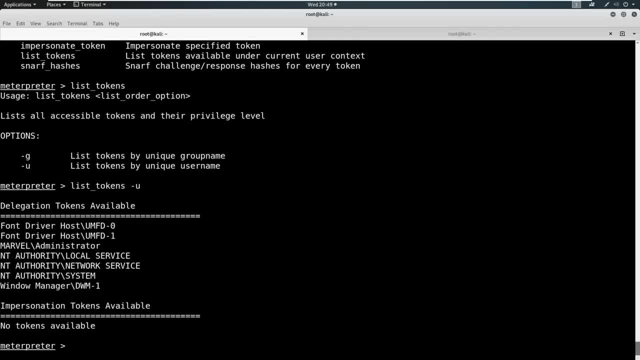 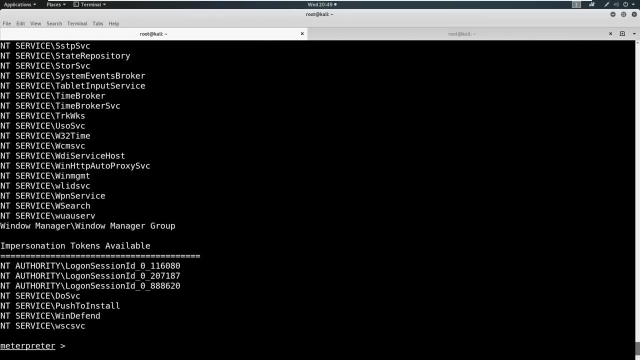 first, however, it is possible that to look through the the group information and see if there's any, and see if we have a member of domain admins, for example, that we can impersonate. if you look through here, we'd be looking for- let's see for marvel. 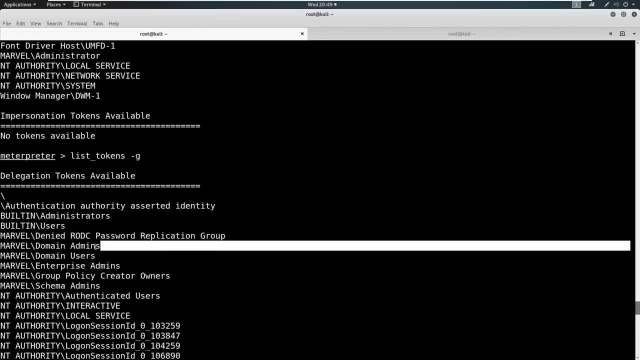 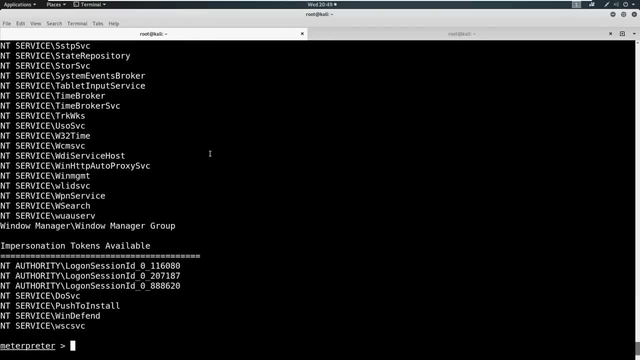 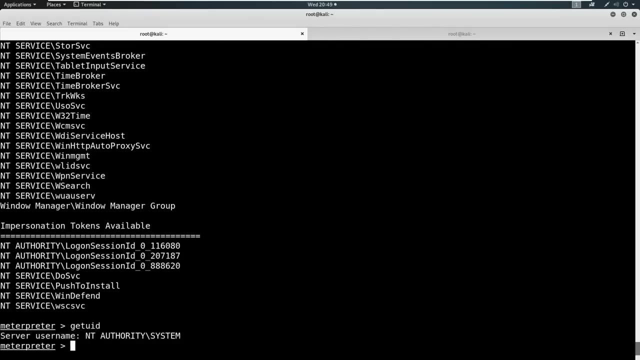 so marvel domain admin does belong to one of these users that's sitting in here. we know it's marvel administrator, okay. so again we say: get uid. and you see right now that we are authority system. all we say is: impersonate underscore token. you can hit tab and then we're going to impersonate. 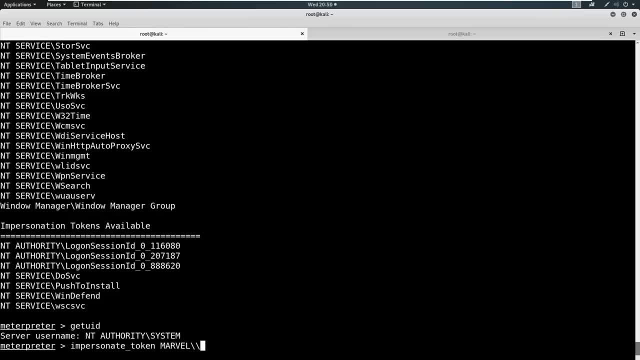 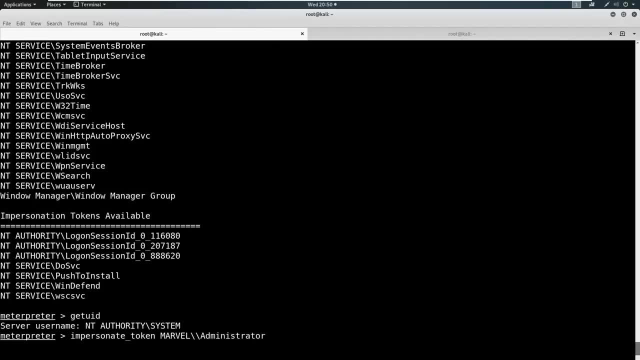 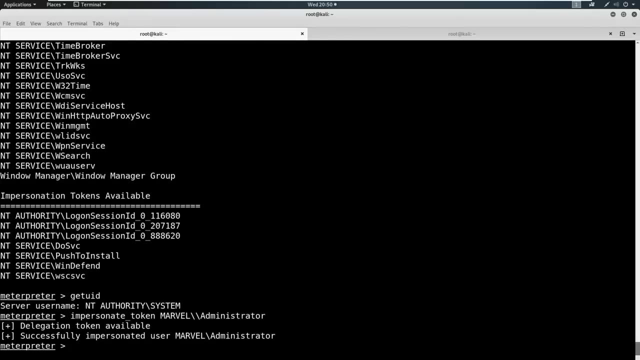 the token of marvel and there is escaping, so we have to do two of these slashes here and then we'll just say administrator, okay, and it says delegation token available. remember, it's a delegation token because we were logging in as the administrator, we weren't an impersonate token. 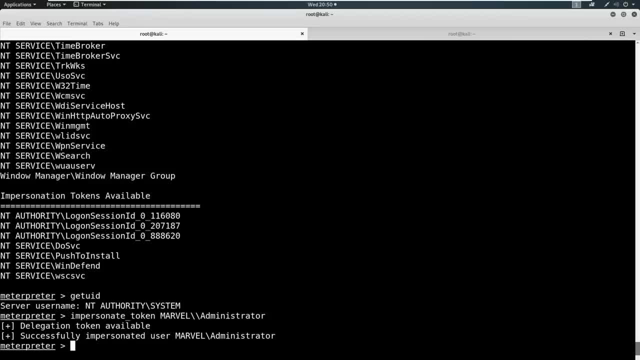 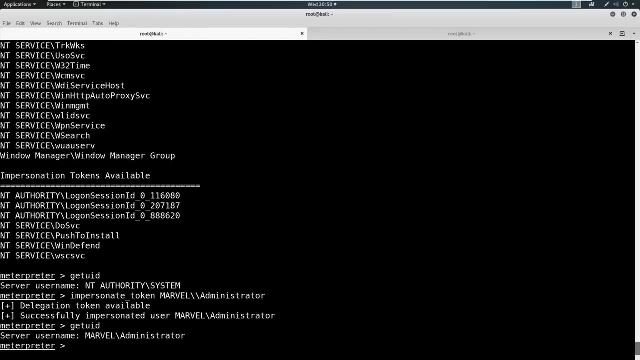 because we were not doing something with like a network drive or a script. so we physically logged in with the administrator. that token is sitting on that computer until the computer is rebooted. so now we have impersonated the administrator. we could say: get uid and it thinks: uh, it thinks we are the administrator. we could type in shell and now we're at a command. 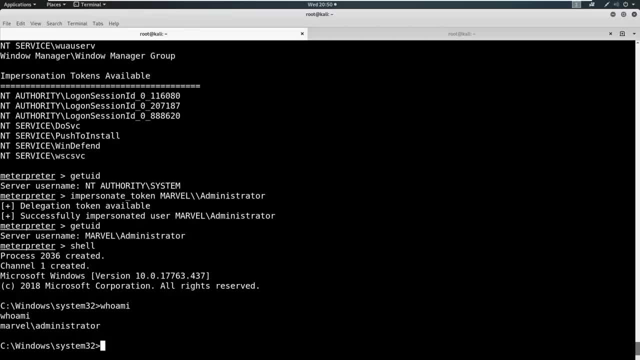 prompt we say who am i and it says you're marvel administrator. so every command that i run from this point on looks like i am marvel administrator. i am doing impersonation here. um, basically this is a path to domain admin. we have accomplished that. we've stolen a domain admin account. 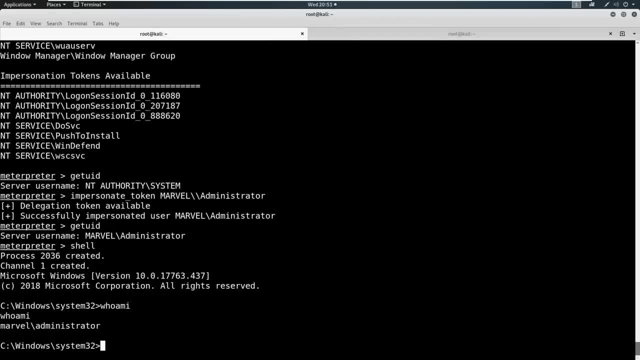 and we can start getting malicious with it. if we want, we can change the password. you wouldn't probably do that on an assessment unless you have the permission to do it. you can try to run net commands and see: now a good, a good environment- and they're starting to do this now- would prevent 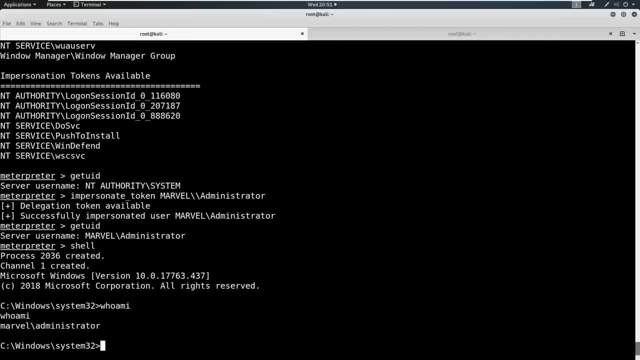 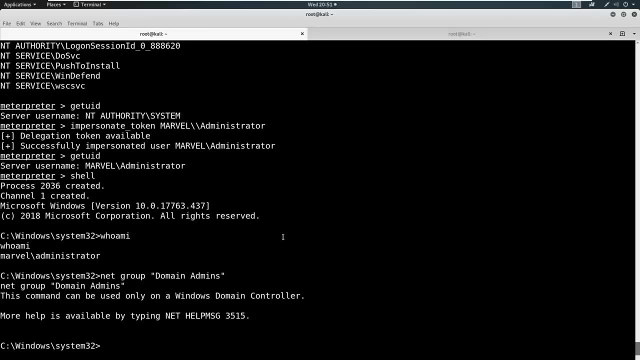 net commands from being run, um net commands that affect the domain from being run outside of a domain controller. so we can try to run something like net group to see all the domain admins and you can see this command can only be used on a windows domain controller. that's a good feature. 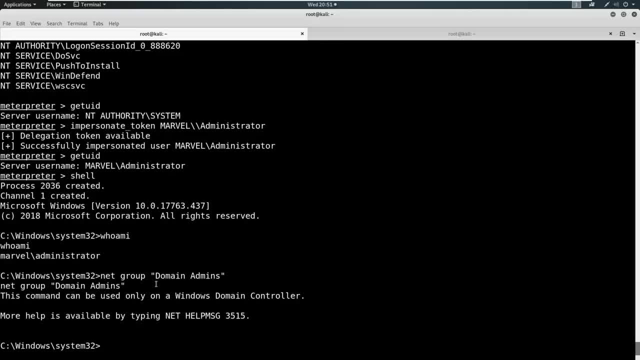 sometimes we can sit here and we can just add a new user to the domain admins and use that with a password that we know, because at this point we don't know the password, we don't know the password for the marvel administrator. we just know that we are the marvel administrator right now, so we can. 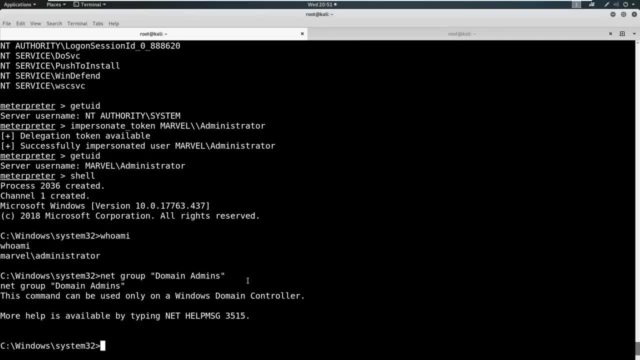 make an account if the net commands were available, and create a new domain admin account with a password that we know, and then just go log in the domain controller and plant a flag there as well. so this is a very, very nifty feature to know, um, let's take a look at some other things, though. 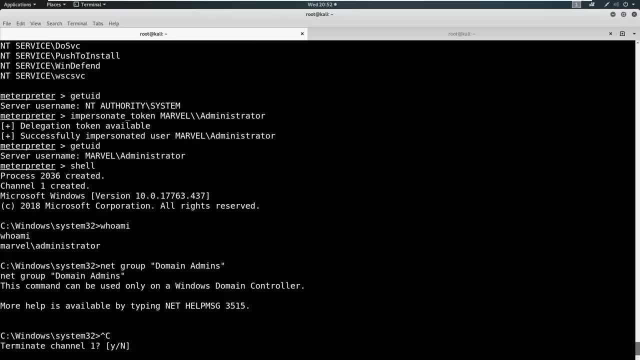 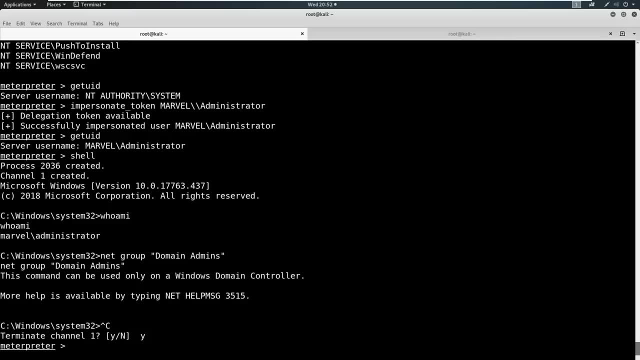 while we're in meterpreter, i do want to show you some things, so we're going to hit ctrl c and terminate this. i need a drink because i've been rambling on. now there are a couple of other tools that we can load in. actually, if we type in load, 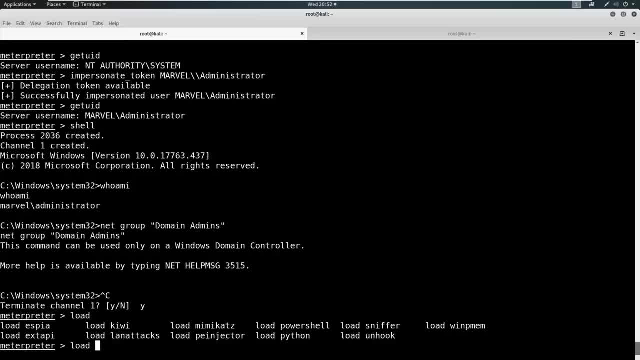 and we just hit tab twice. you can see all the other things here that we can load in. we can load in powershell- python, mimi cats, kiwi, and i encourage you to go into a meterpreter and load in a tool called mimi cats and i encourage you to go into a meterpreter and 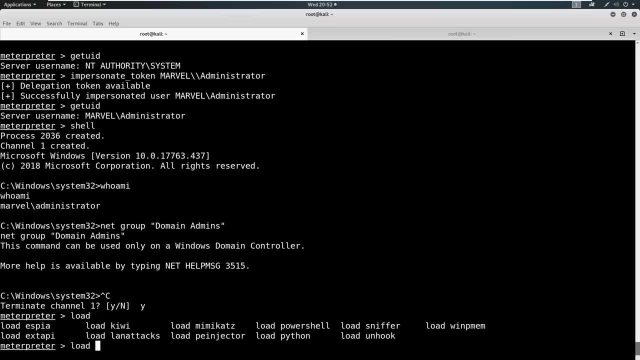 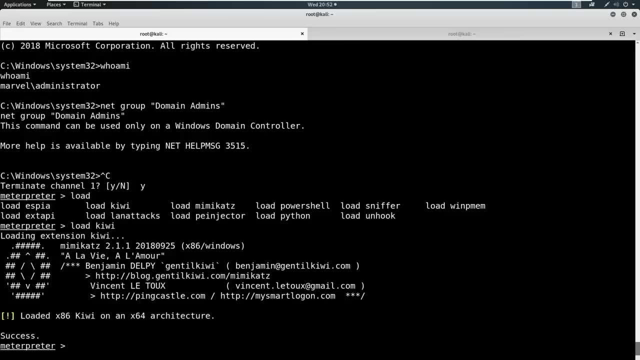 shell load all these and figure out what they all do. so when we're on a 64-bit architecture we can load Kiwi. now we are not on a 64-bit shell, so you're gonna see it says: loaded x86 Kiwi on x64 architecture. so this is not gonna. 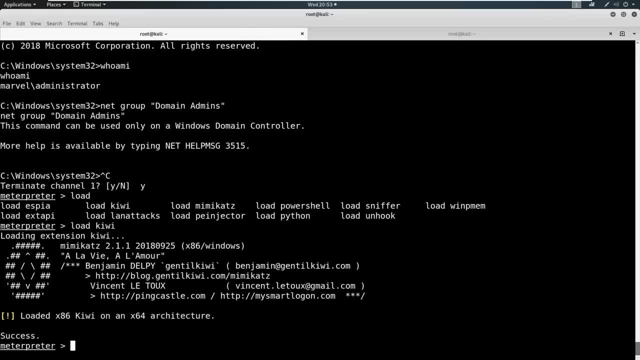 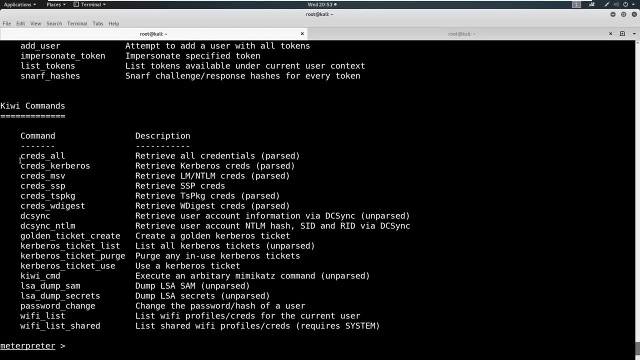 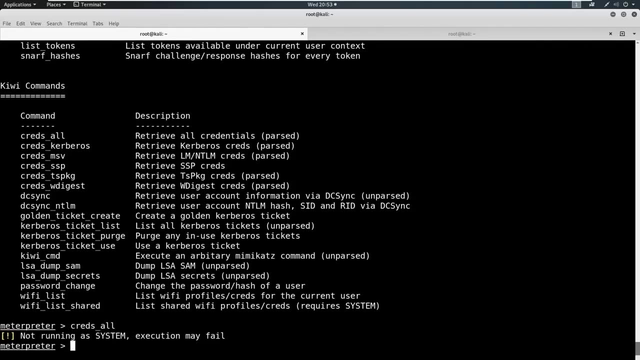 actually work. so if we look at it here and we could say: help, and one of my favorite commands for Kiwi is just to dump the creds all right here on the top, we say: creds all not running a system. okay, so we're still running as the 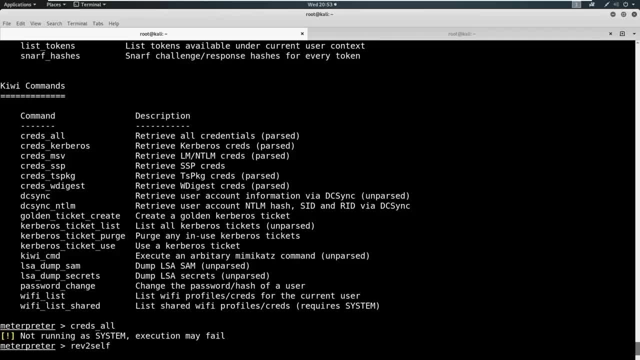 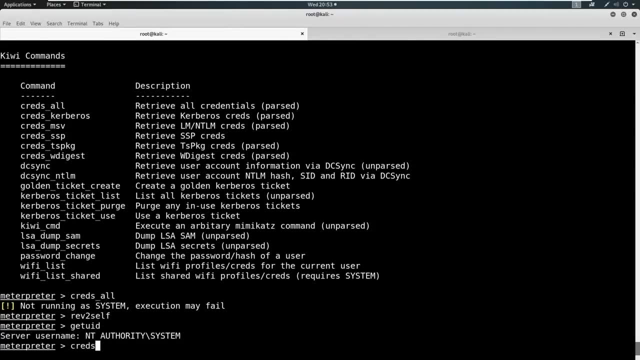 domain administrator. we could do rev to self and that should get us back to system. this is reverts back to who we were to begin with. okay, now we can try creds all and you're gonna see that it doesn't dump anything. there's, it's not. 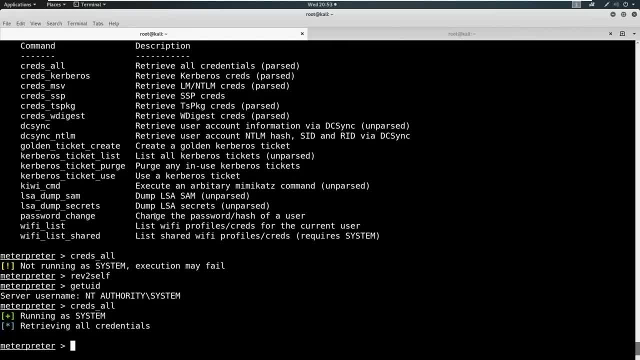 gonna dump anything because of the system and it's not gonna dump anything because we're not running in the right architecture. but do take a look at what is dumpable in here. right, Kerberos? you got the W digest. you can do golden ticket attacks, which we're not going to get to in this course, but this is 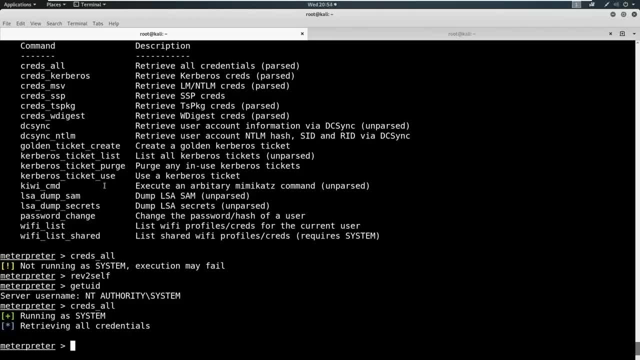 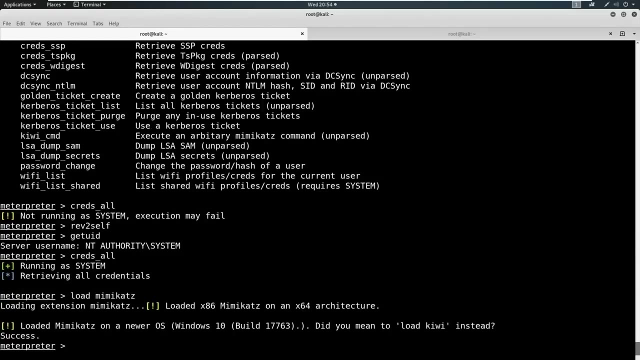 another common. if there's a top 10 golden tickets, probably in the top 10 we've got Wi-Fi profile lists and credentials. the LSA sometimes has useful information in it, so these are are good to look at. now for a 32-bit system and a 32-bit shell, we could load Mimi cats and you can see that it. 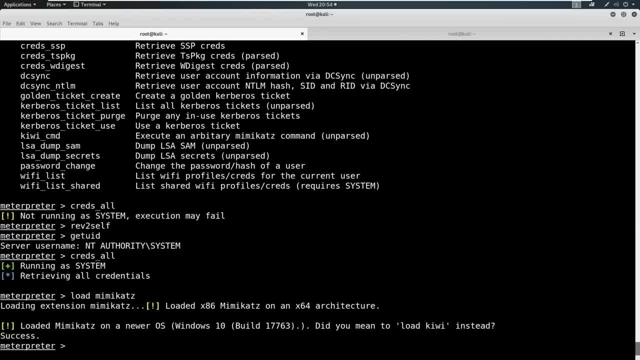 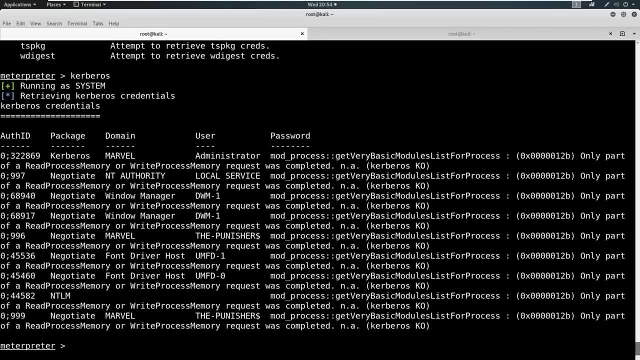 doesn't like that. we're running on a newer system. this is typically for older systems. we could say help again, but we can start just typing in things like Kerberos, okay. well, we didn't get anything really useful out of here, and again it plays into the the issue that we're having. so 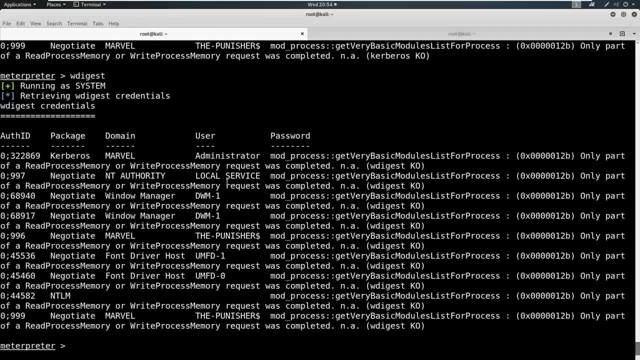 now that I've shown you everything, I may go back. once I get everything shown to you, I'll go back in and and try to migrate to a process, and if we, if we fail the computer, we failed the computer. okay, so from here, one thing that we can do that's useful as well, is we can 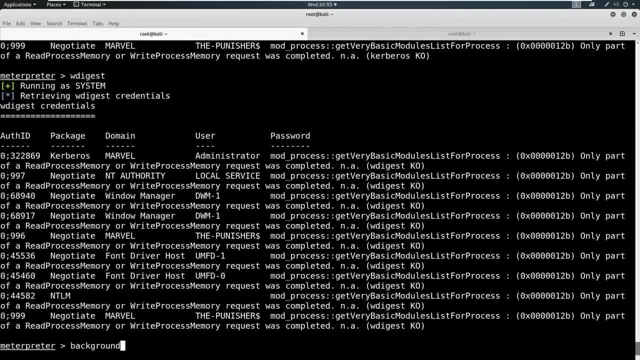 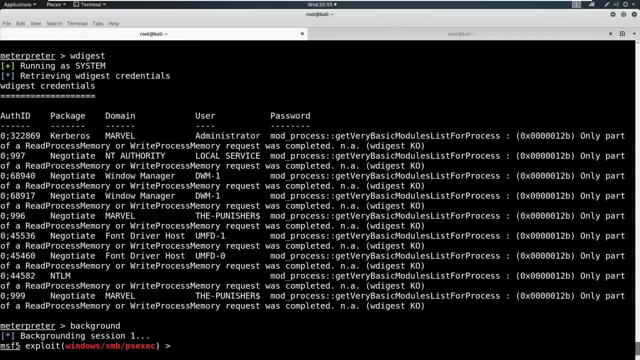 background. right. so I showed you that earlier by just doing it on my own. we just type background and background this into a session. if you notice now, it puts us into it, puts us back into a meter per or a metasploit area so we can pick modules. that session is still running. if we type in sessions, it's. 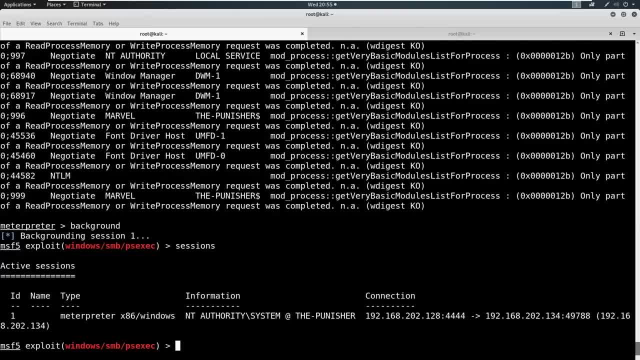 still running in the background and what we can do with it is we can use that session in other places. one of my favorite things to do on like hack the box, capture the flag, is to use a tool called the local exploit suggestor- suggestor, and that is a. 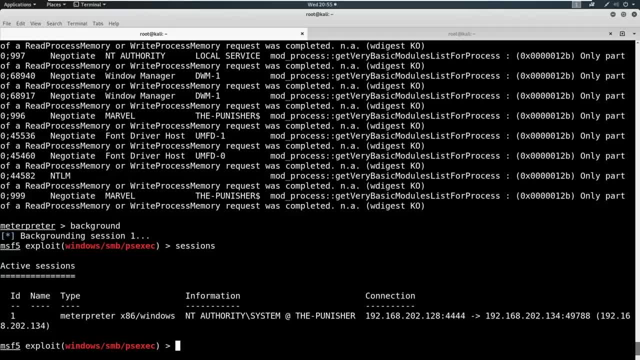 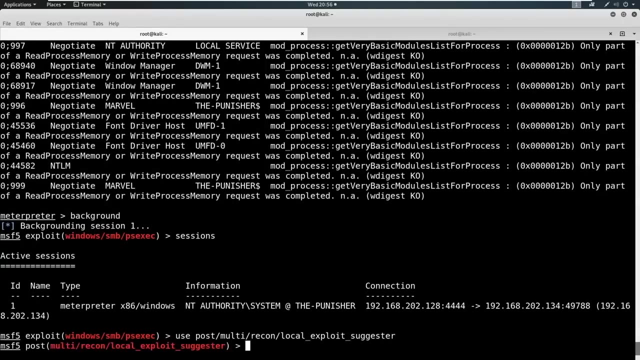 post command, meaning we have already exploited. so this is after the fact, so we can search for that. but I'll just type it out here. we say use- and it is post multi recon, local exploit suggestor like that, okay, and then we'll just type in options. 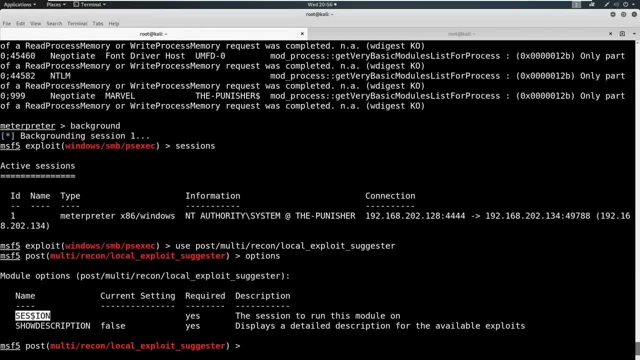 and you're going to see that it asks for a session and that's all it needs. and now I don't know if this is actually going to work because of the mismatch we have, but I do want to show it to you. so let's just say: set session one, and I'll 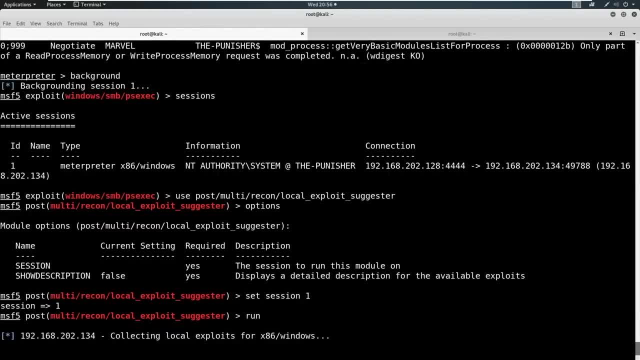 run it and now it's collecting local exploits for x86 windows. that's really not the case, right, because we have 64 bit windows, so this may give us some false positives here. but what it does- is it just here, it just puts us in this- is it collects everything that may be an exploit, and this leads to easy win a lot of times, like 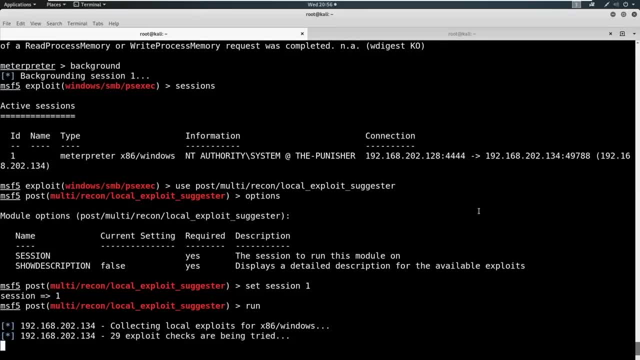 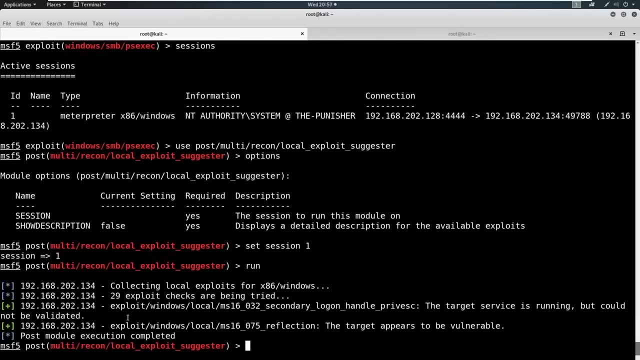 i said on capture the flag, or even if you're in a situation where you're not able to escalate to system for whatever reason in your environment, what you can do is it suggested two different situations here? right, so we can try to run this exploit against the session. this priv ask here. 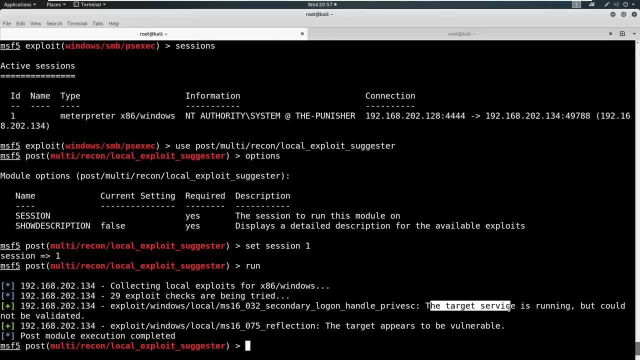 or this priv ask here. it says it thinks it's vulnerable, can't validate it, and this one says it appears to be vulnerable. so we would just say: use, exploit windows and we'd set the session again and try to run it. now i'm going to go ahead and, uh, and take a peek here and see if we can't migrate. 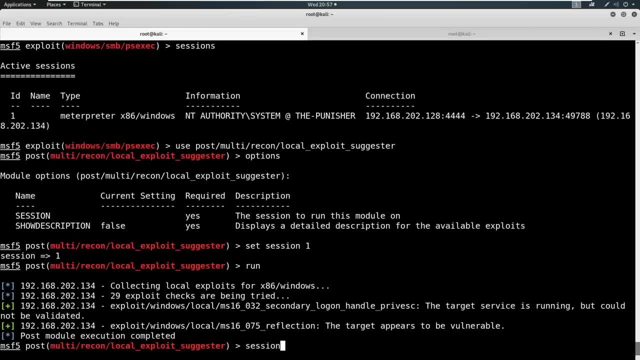 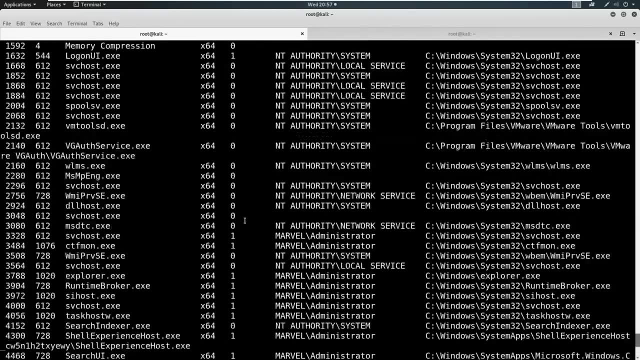 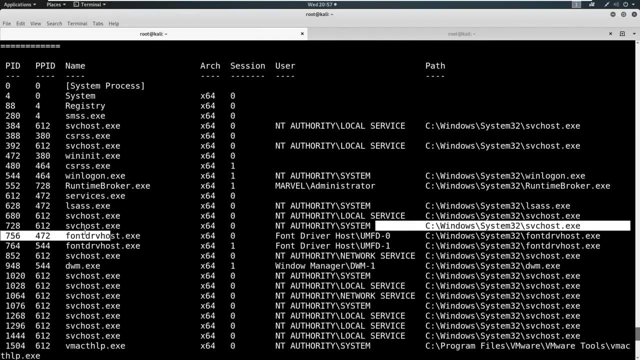 this session. so sessions one. and then let's take a ps again. you want to pick a number, rury you feeling? you feeling like, uh, you're gonna win the lottery here. we've got svc host on 728, i'll let you. i'll let you pick buddy. this is rury's choice. 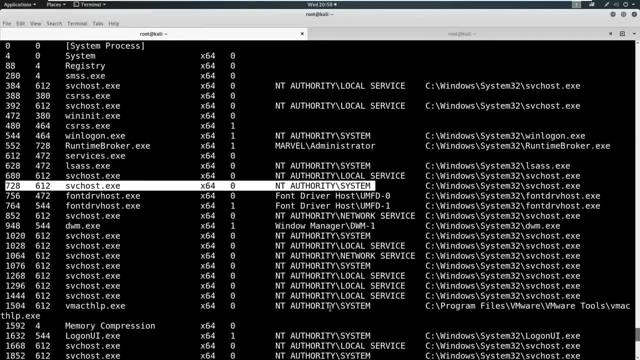 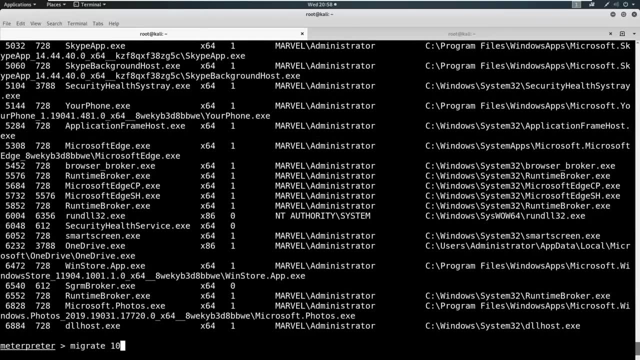 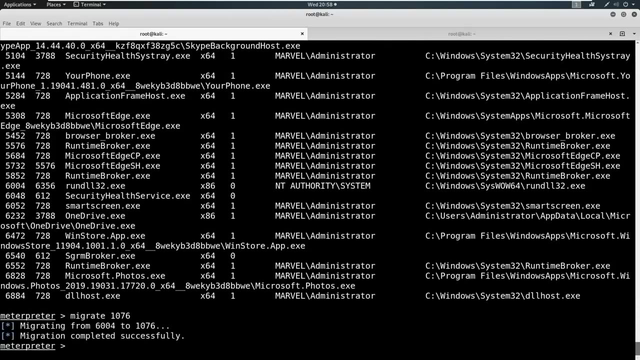 give me a number: 10 76. we're picking 10 10 76. we're picking 10 10 76. all right, here we go for all the marbles people. it's either gonna make or break our shell. he did it. he did it guys. 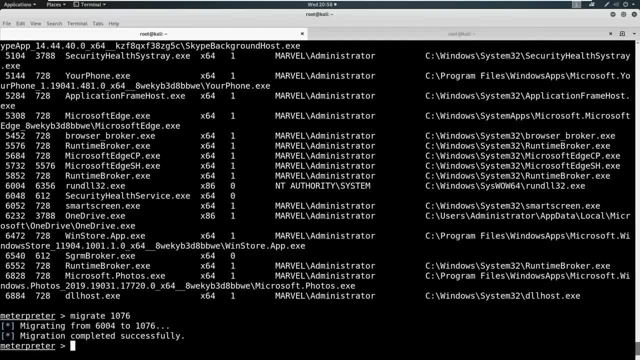 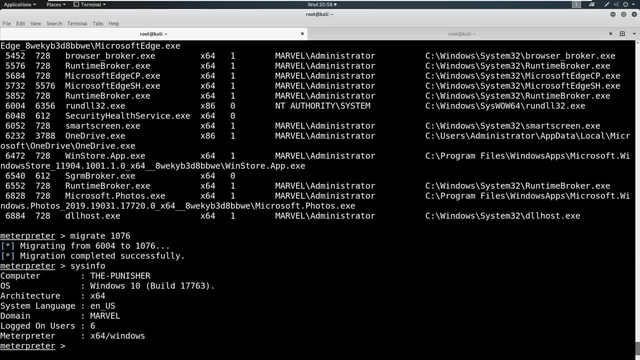 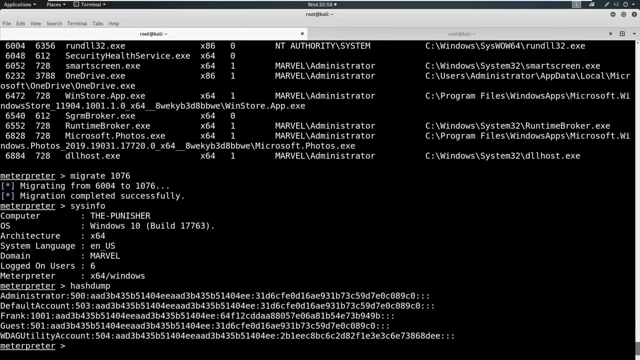 look at that always: trust rury with your, your process. migrations. beautiful, beautiful sir, today you win the internet. all right, sis info. now you see we are on a 64 aliment interpreter with a 64 architecture. now we can do some fun stuff like hash dump. oh shit, look what we just did: we dumped all the hashes. 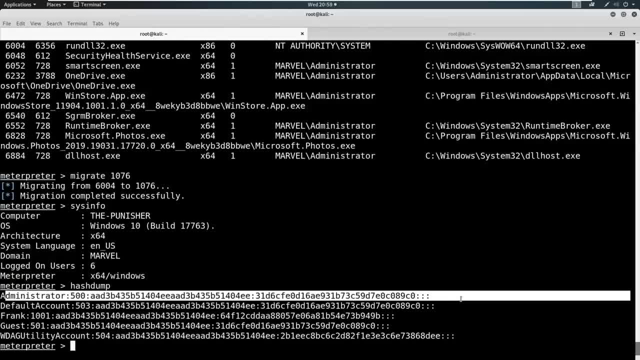 like hash. i mean hash. we propose today spice packs mixed been adjust. this will appear in the same window as we did with port officeапit: comes by default. we actually never said a password or set that up. i don't believe this will happen because we went in and we set up frank originally and this is not. these are all local accounts. these. 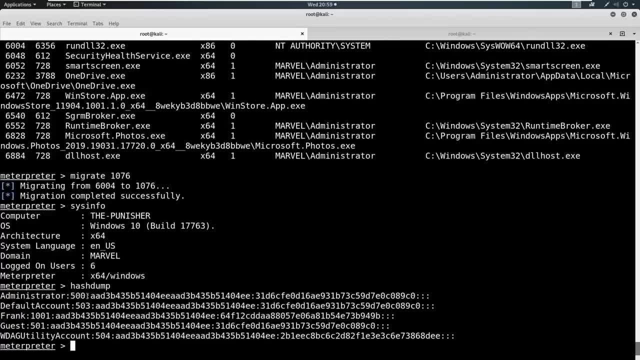 are not tied to active directory, but we have hashes here so we can take these hashes and try to capture them. we can also take these hashes and try to pass them around the network and we can use something like crack map exec to do that, and i'll show you how to do that. 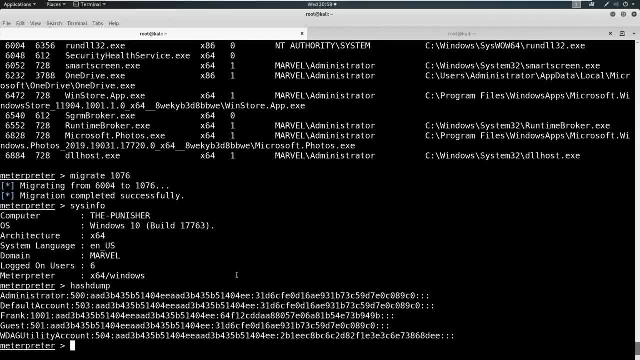 but let me, let me tell you a a situation where this comes in handy. now. think about an environment- and this has happened to me many times. think about an environment where they have a lot of computers and they take the same image from every computer and they use it right. they image the all their. 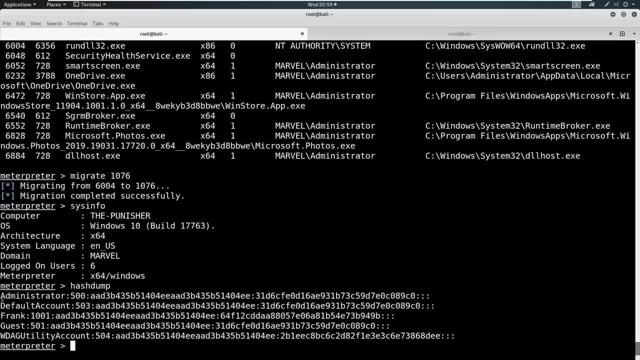 computers are the same image, the same base image. well, that same base image is going to have the same administrator account, so i don't even have to know a active directory account to log into that computer. i'm sitting here logging in a system to every computer in. 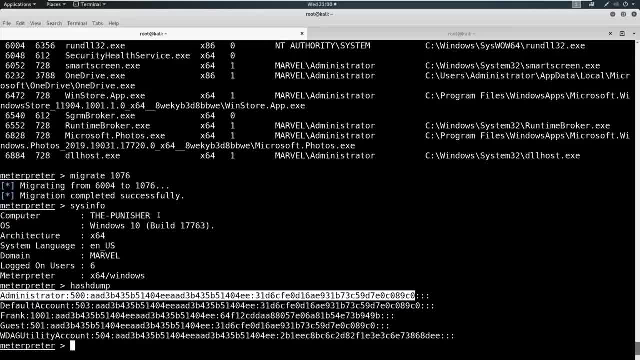 that network. it's only going to be a matter of time before i get credentials, or i do token impersonation, or i find something in a file that i shouldn't be seeing, or if i get onto like an it account and get all the passwords. so this is, this is win a lot of the times. so there are two. 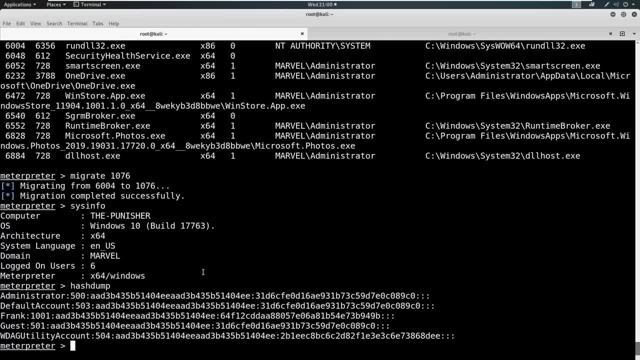 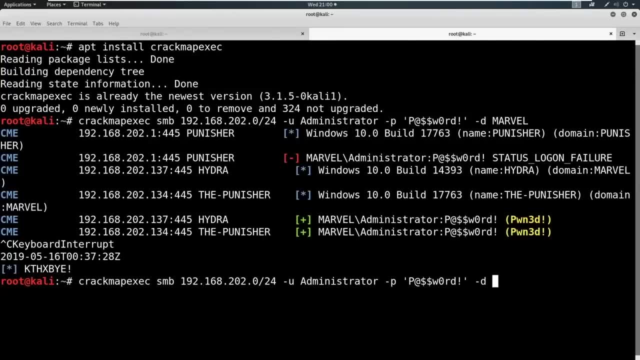 different ways that we can do this. basically, what we can do is we could use crack map. let's go back up here. if we hit tab up, we'll delete marvel, and i don't know if this is going to work, so let's try it though. let's capture. 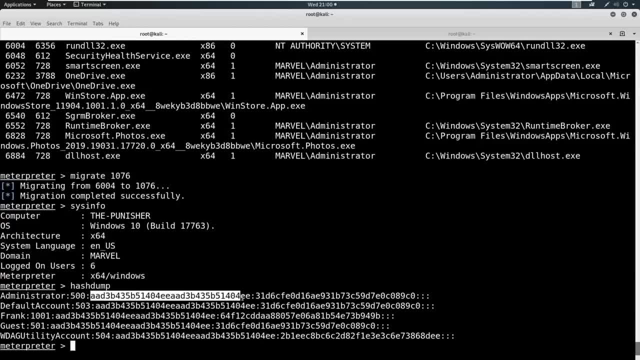 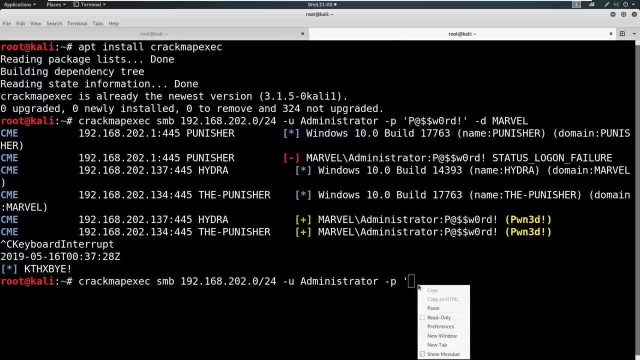 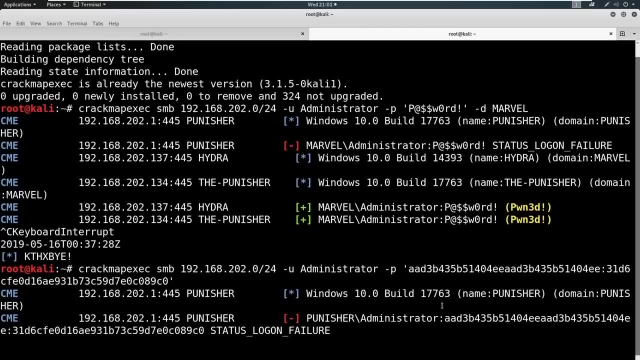 this hash here. you'll start from the a's and bring it all the way over, just like that paste. i'm going to keep the quotes around it. we may need to remove the quote. it might not recognize it as a hash. it doesn't look it's. 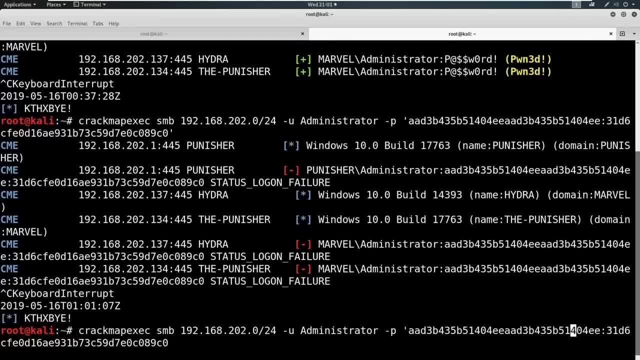 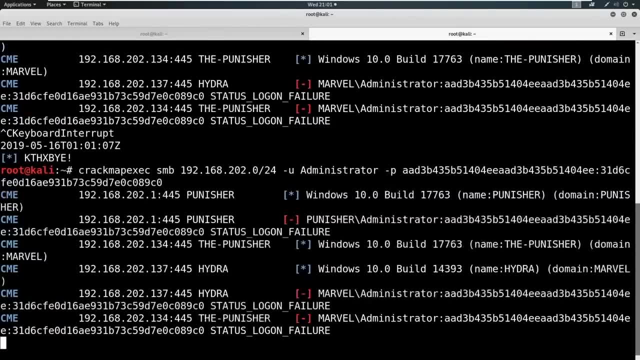 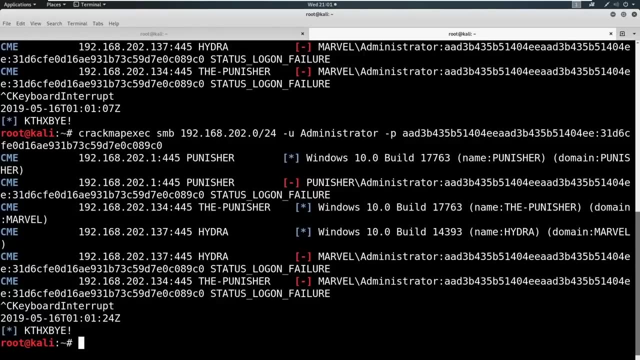 recognizing it and, again, i wasn't getting these working. but this is the methodology that you would use to try to log in, so you would try to pass this hash around and you don't even know, need to know the, the password, to do this right. hey, thanks, eric, i really appreciate that. 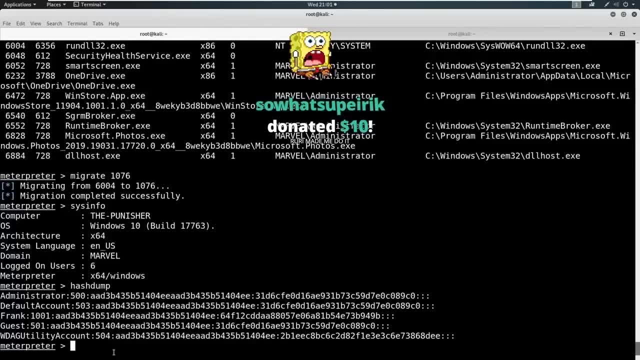 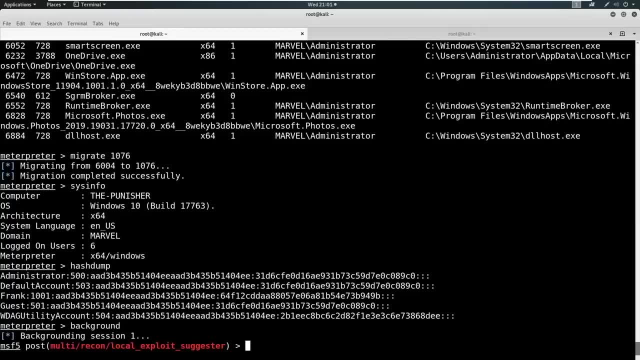 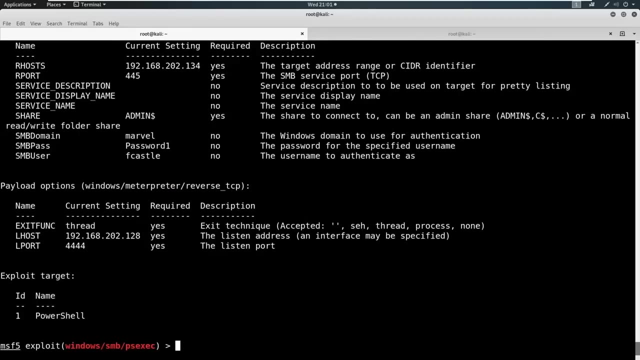 so another method, if we background here is we can actually use ps exec as well. so what we would do is we'd say use exploit, windows, smb, ps exec, again like this: let's look at our options. okay, we'll keep the machine because this is the machine we attacked. we'll say admin or 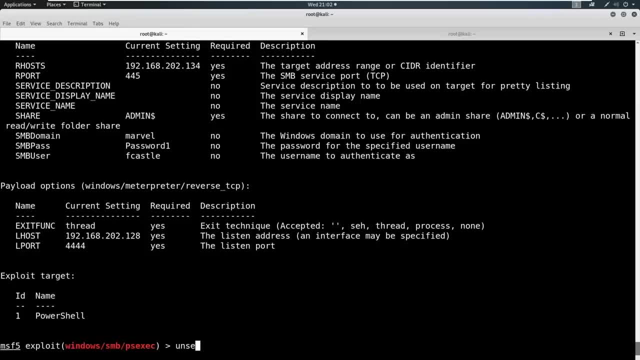 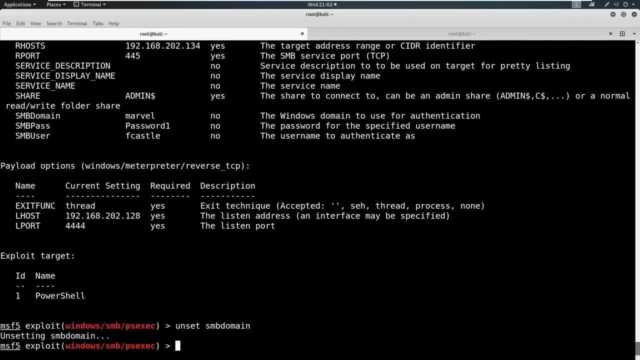 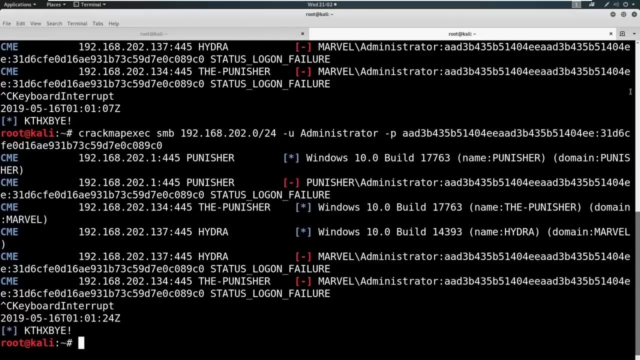 whatever, and we're going to use the machine we attacked and we're going to use the machine we here. but let's say unset smb domain and somebody said to use the dash h. you are absolutely correct. i completely forgot to do that. so one second that could be the whole issue entirely. 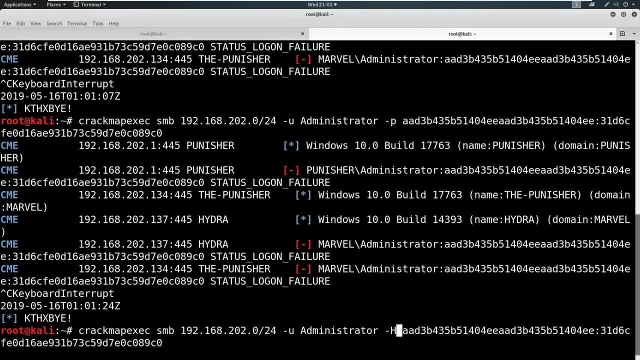 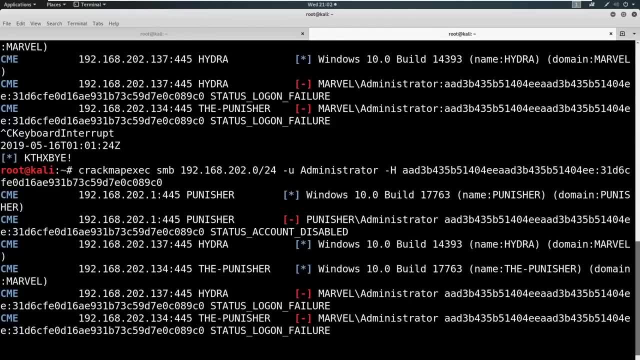 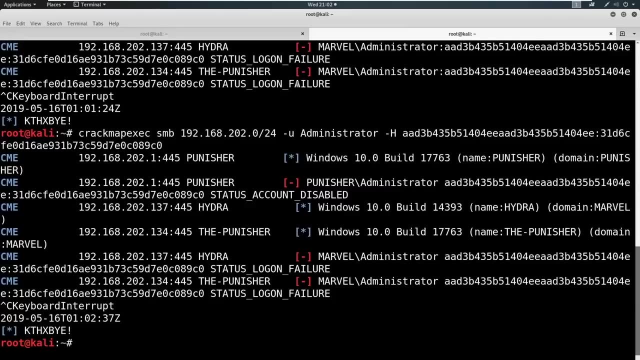 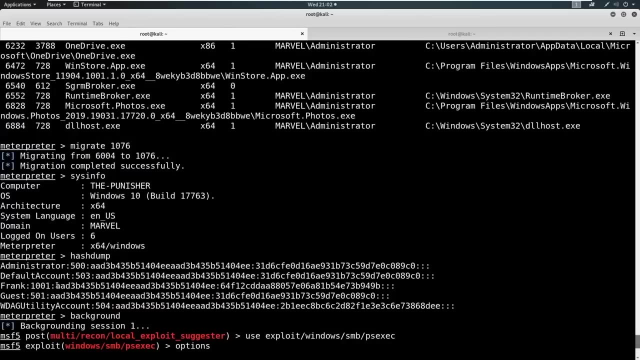 thank you, solo. i messed up my syntax. see if it works. still not getting it. i don't know if this account is active. it would probably be better to try it with the frank account. we can try it with the frank account. let's grab frank instead of administrator. 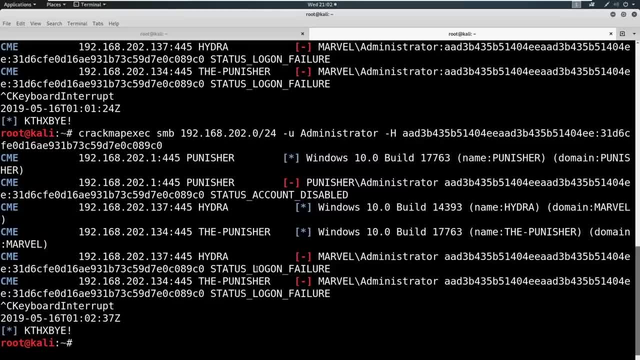 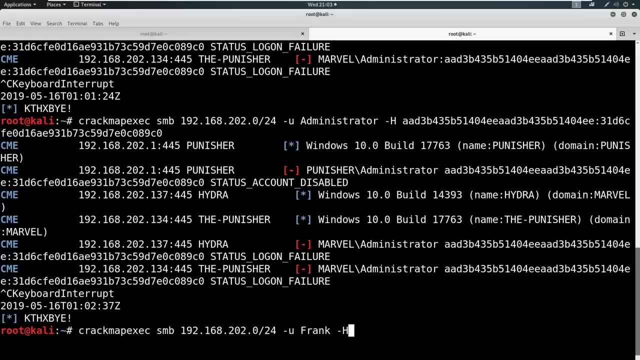 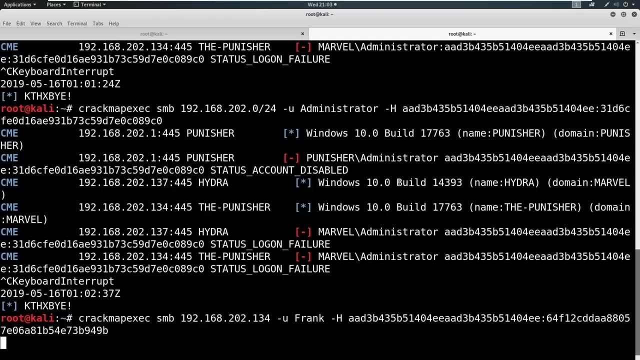 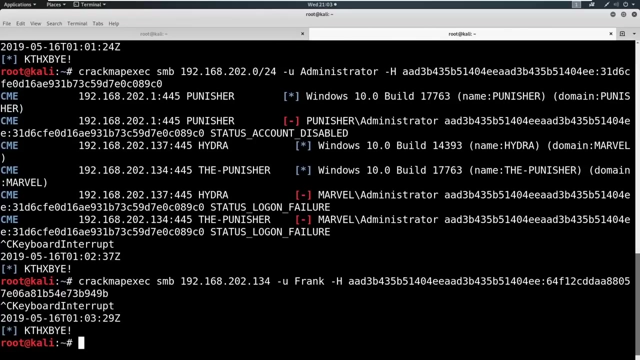 and let's actually just point it right at 134, 134, let's see if it works. 134, 166, 167, 168, 166, 168, 168, 169, 169, 169, 169, 1610 and not getting a response? all right, let's try. let's try sweeping in the network again one more time with it. 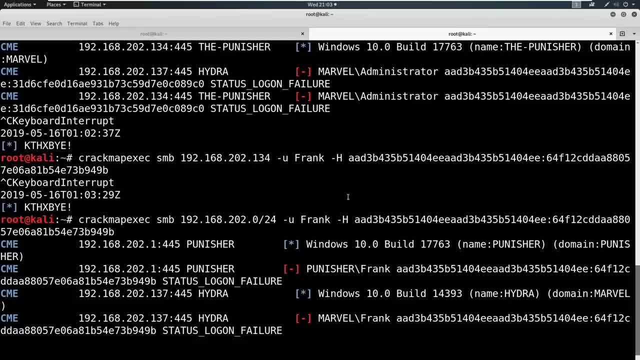 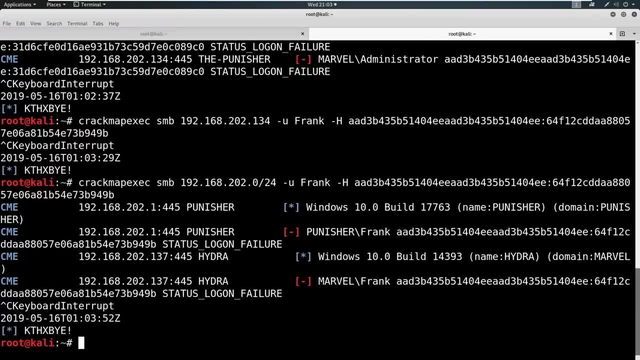 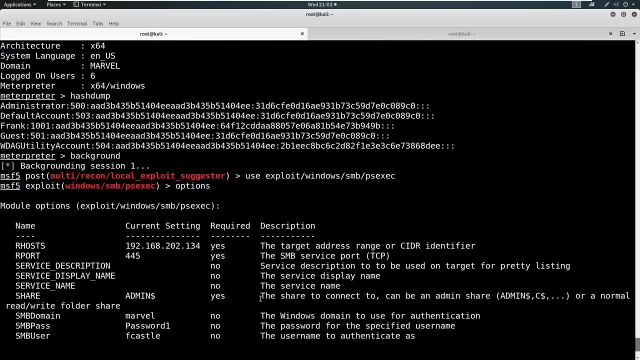 it's not responding on 134, and that's okay. it could be that it's actually connecting and it's having issues, um, so let's just kill that. but that's one method. that's one method right there to pass that that hash around. uh, the other method is with ps exec. so we're in here, right. 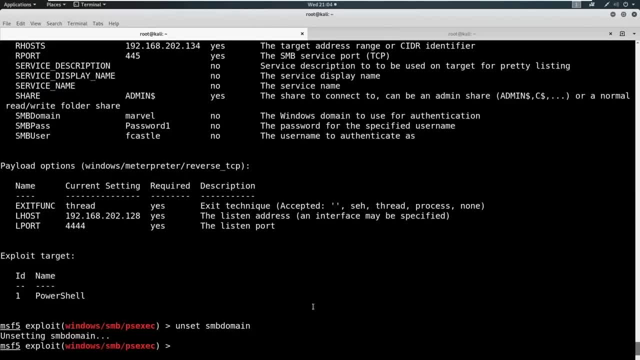 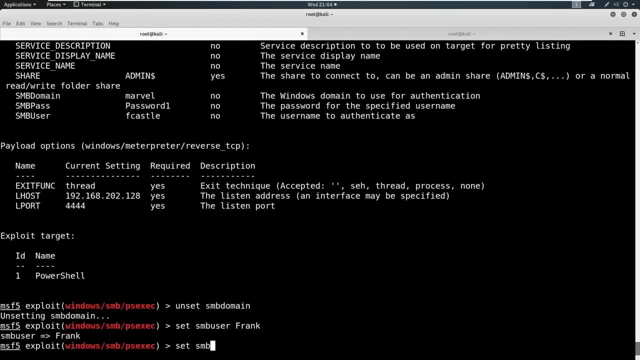 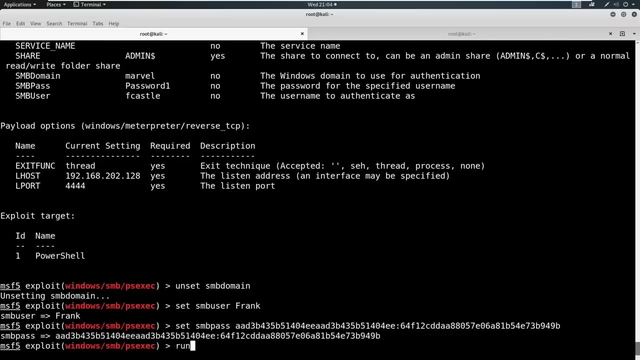 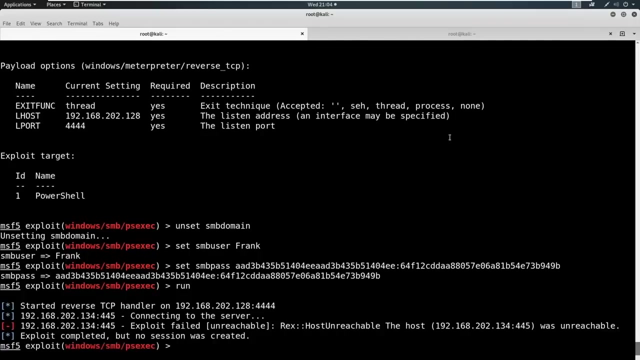 i unset the smb domain, so we're going to take that off. let's set the smb user to frank and then let's set the smb pass as that hash there, and and and. we're going to try running this. yeah, we're getting host unreachable. we may have lost the connection. 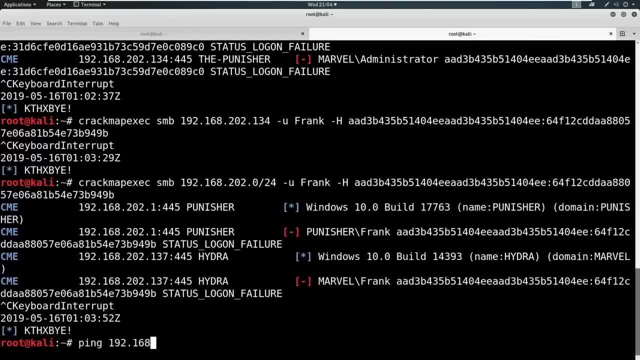 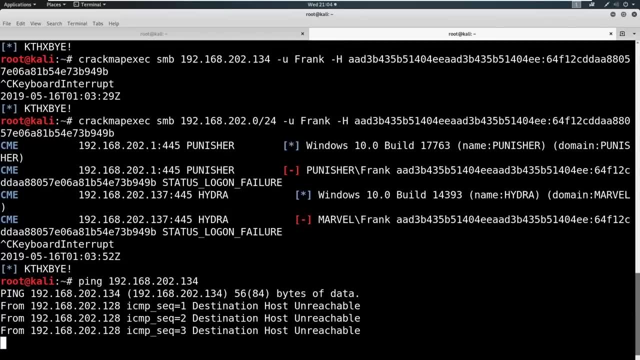 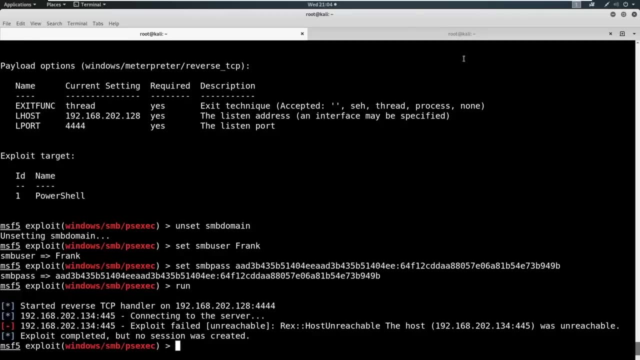 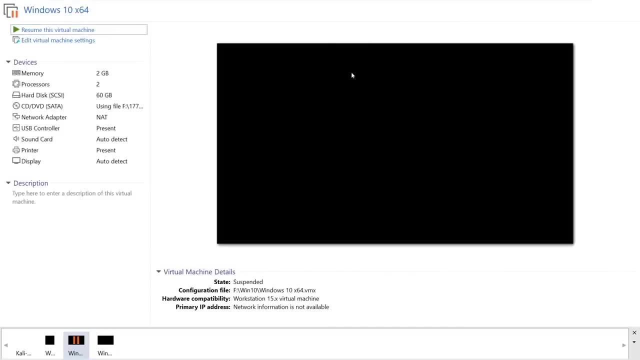 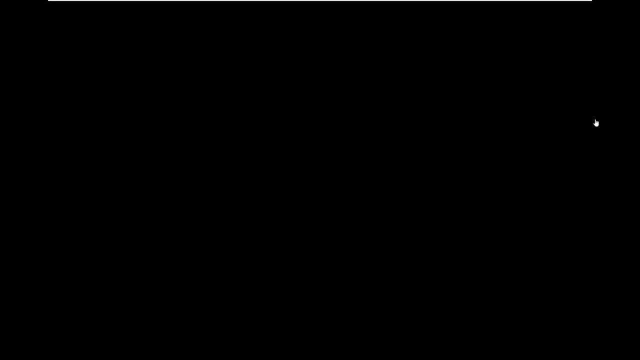 that's a rip just when we were getting our mojo. that's okay, we'll reboot it. may have fallen asleep and i'm yeah. it paused itself. these machines, man. i don't have my settings on right, so the machine paused itself. all right, let's try it again. 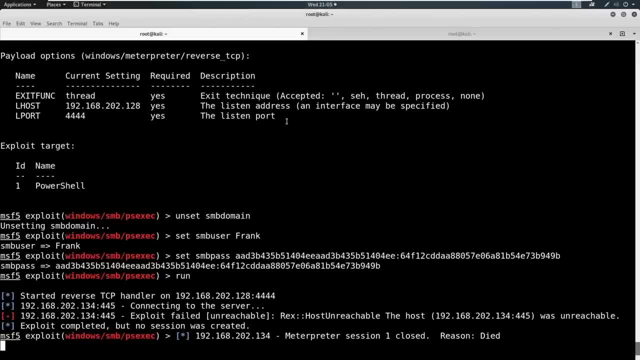 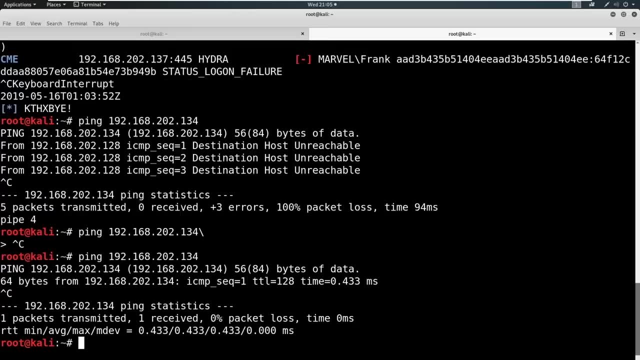 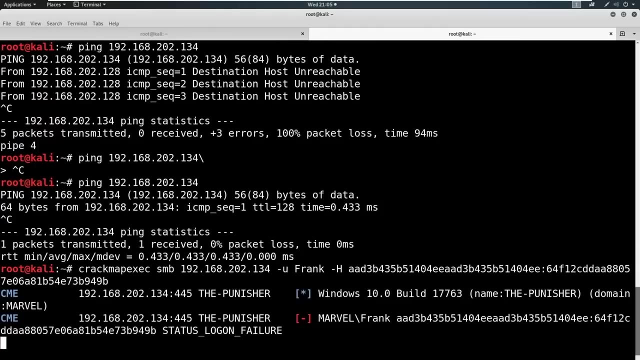 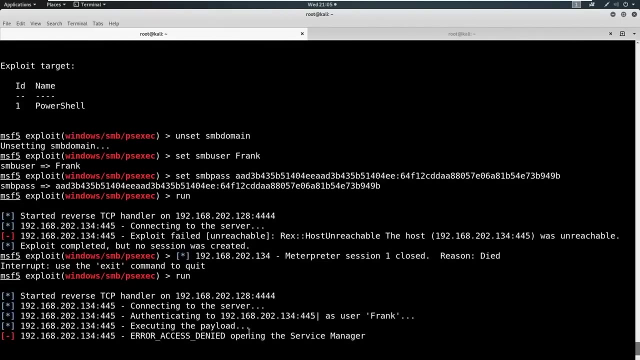 see we lost our, our shell there as well. oops, okay, it's back to life. let's try crack map one more time. 134 still got a login failure and we could try with ps exec as well. now that it's up, access denied here, we could try setting the target to something else. 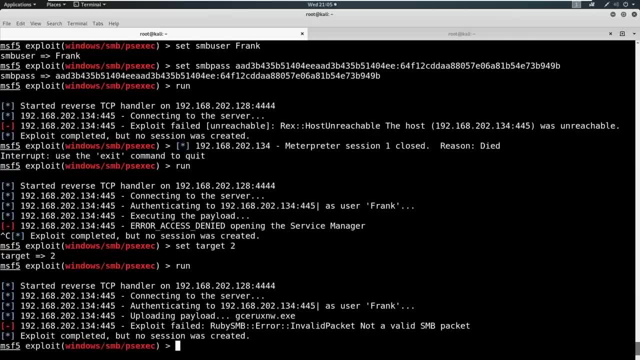 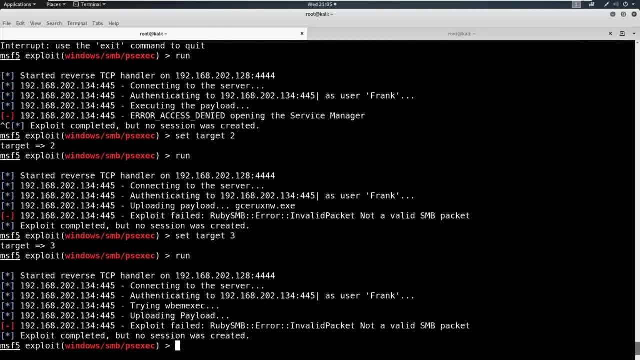 so it's connecting, but it's not. it's not able to execute. so so it's connecting, but it's not, it's not able to execute. so it's connecting, but it's not. it's not able to execute. So the question was asked. we disabled Windows Defenders or anything else. 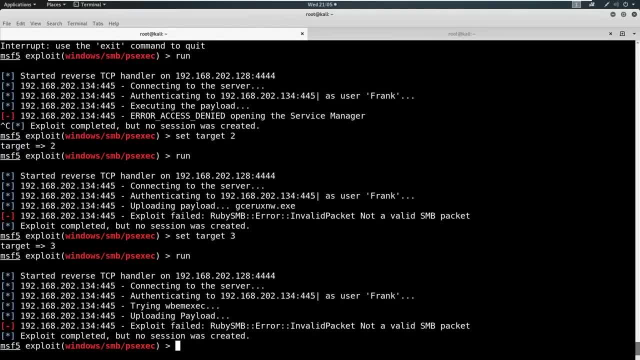 We created a scans folder and made the user domain admin, but I think you're already passed out. if you're on the Windows Defender, What's up Sick in the Mind? All right, everybody. So this is just a lesson. I'm going to pause it here because we're already at 9.06.. 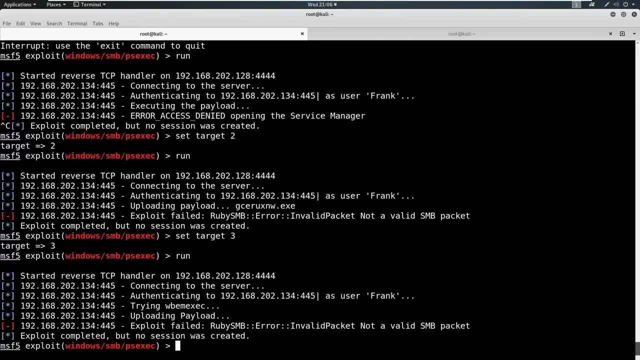 This is a lesson and what you need to take away from it is what happens with credentials from LLMNR poisoning- that we can do these PSExec attacks we can do, token impersonation we can do, pass the hash. we don't even have to have the hash or the account cracked. we 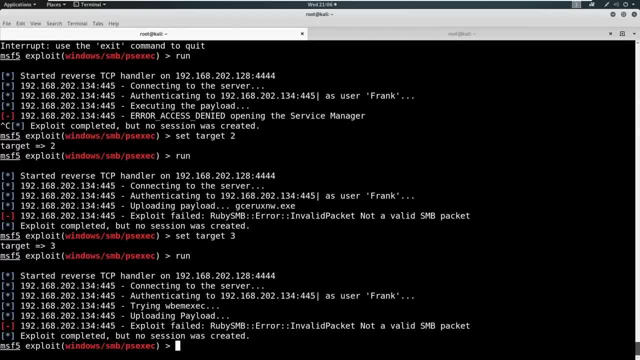 can pass the hash of what we gather for local accounts and we can take the accounts with CrackMapExec as well and pass them around with a cracked password and see where we can log in SMB. majority of the time, bad passwords, along with SMB, are going to be the easiest. 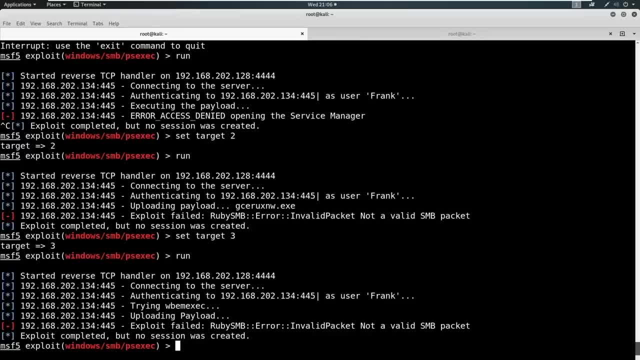 way you're getting around a network and getting your win. If you have long, complex passwords and you don't have SMB in your network, you're going to make it a lot harder on us as a pen tester. So, with that being said, many of you are asking about NTLM Relay. 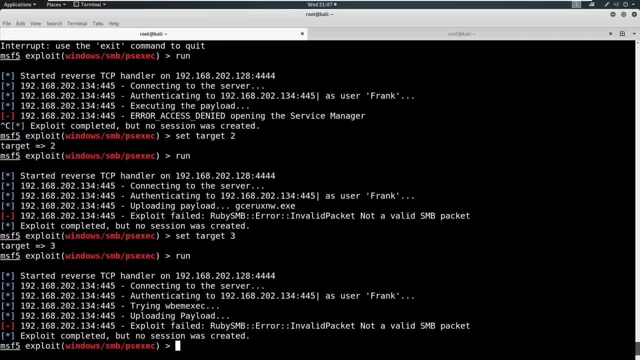 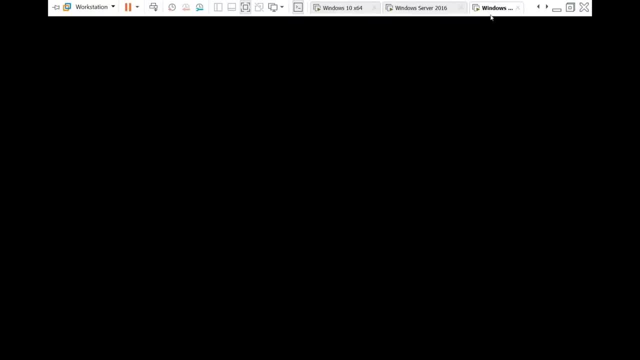 That is going to be the next thing we're going to cover and then we're going to call it a night, So let's go ahead and do that. Now we're going to have to do some setup. I've got 2016 server running. we've got Windows 10 running here, and am I missing a 10 machine? 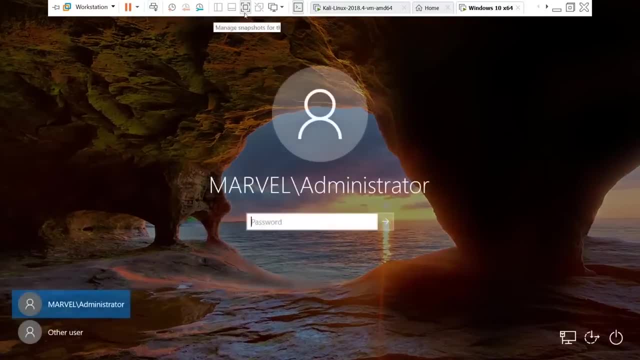 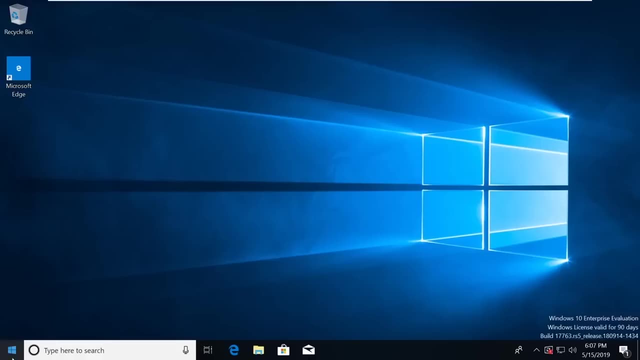 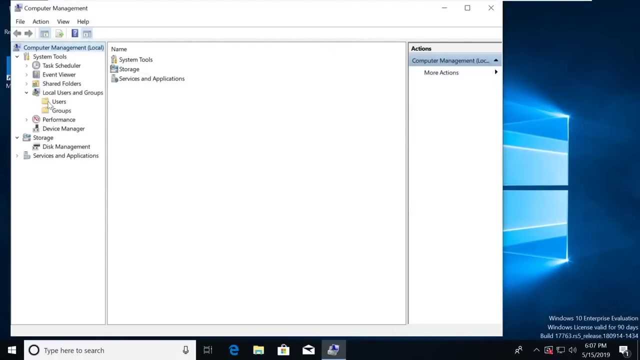 I've got. let's see which one this is. This is Marvel Administrator. okay, this is the other one. So, Windows 10 machine. we are logged in and who are we? Okay, so, yes, this is the right one. 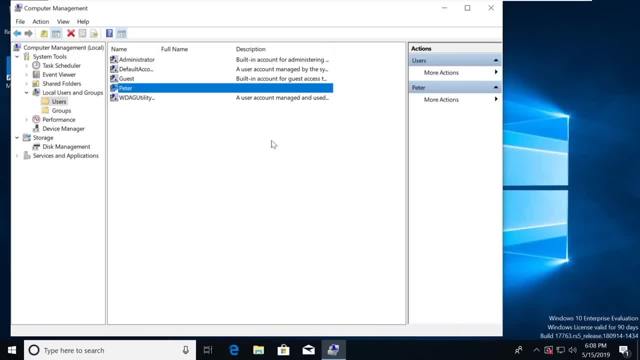 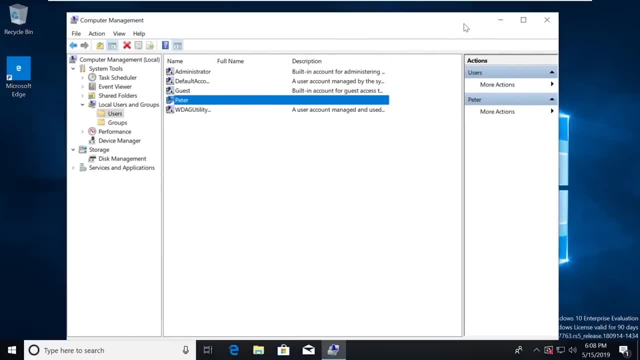 So we've got a. we've got another computer here. this is going to be Spider-Man's computer. we've got Peter Parker. I've just created a local account at this point for Peter. so what we're going to do is we're going to set up a Relay. 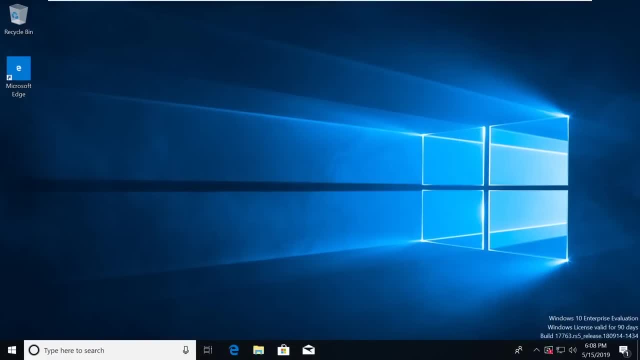 Relay attack. Now, a Relay attack is where we are capturing the LLMNR hashes and, instead of taking them offline and cracking them, we're actually going to relay them to another machine and try to get information off of it. So here's what we're going to do. 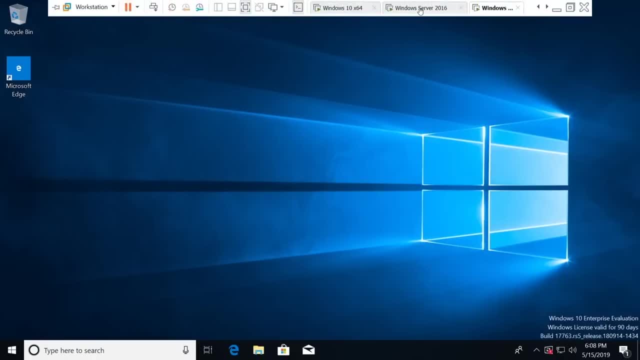 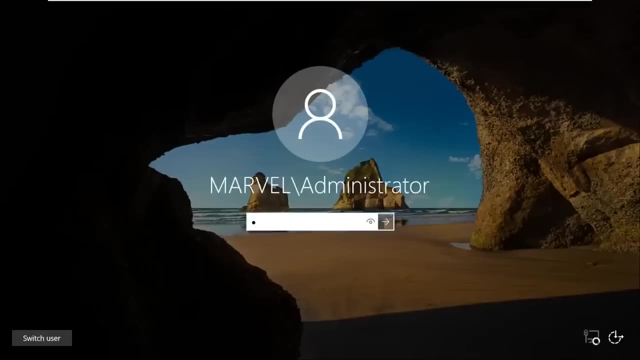 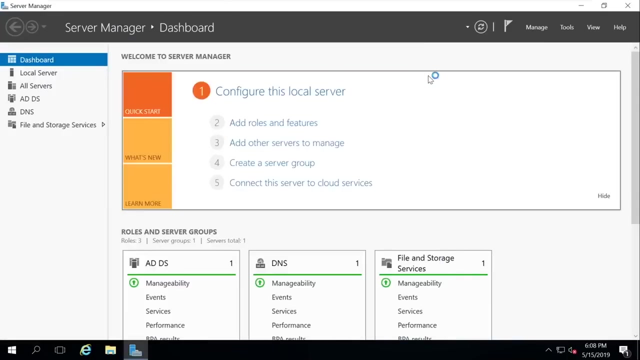 First things first. we need to go on to the Windows server. So let's get there, Let's log in as the administrator. Okay, And I've got all this open. I'm just going to close it out. we're going to redo it all. 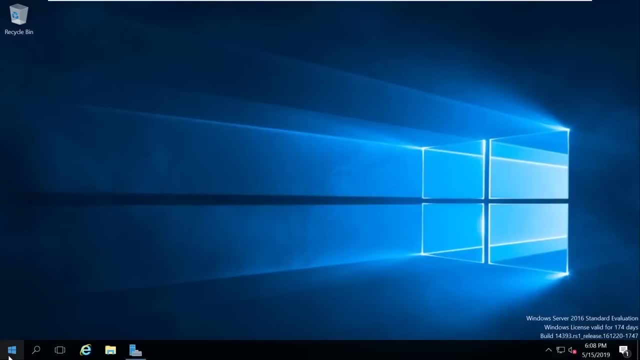 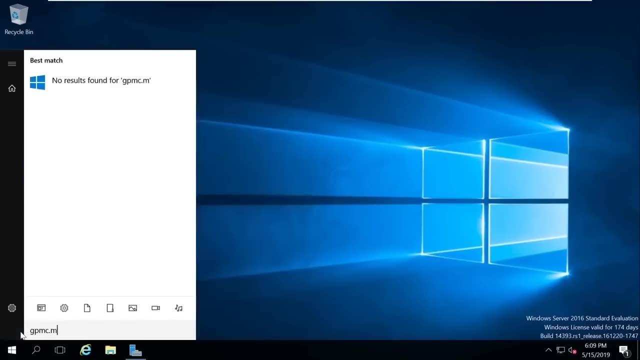 Okay. so what we're going to do is we're going to come into here and we're going to say we're going to start typing gpmcmsc. I'll give you a second to catch up if you need to. 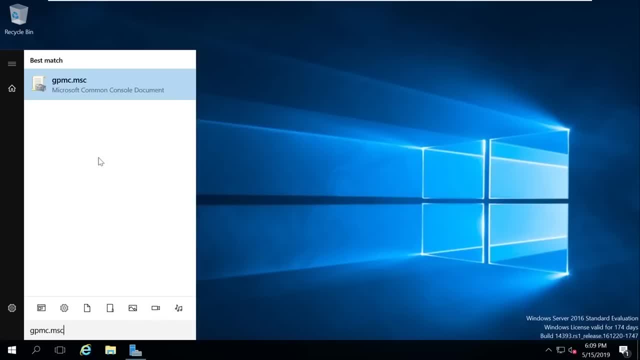 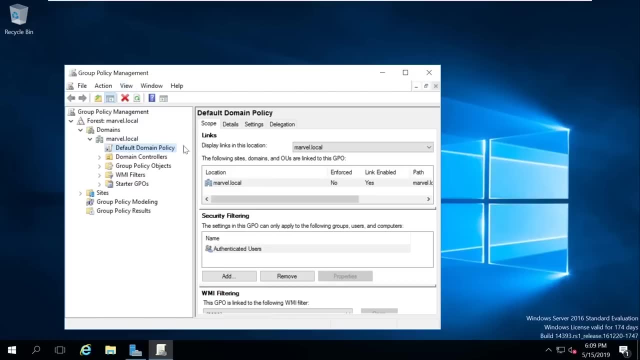 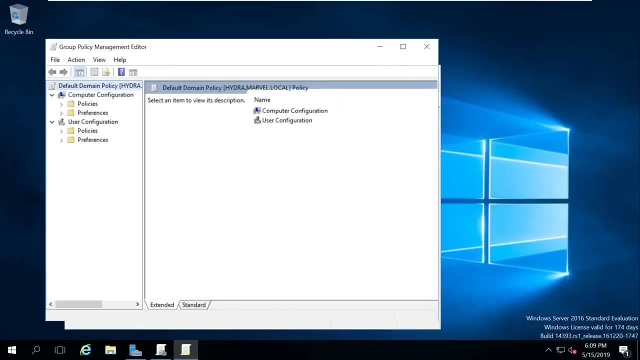 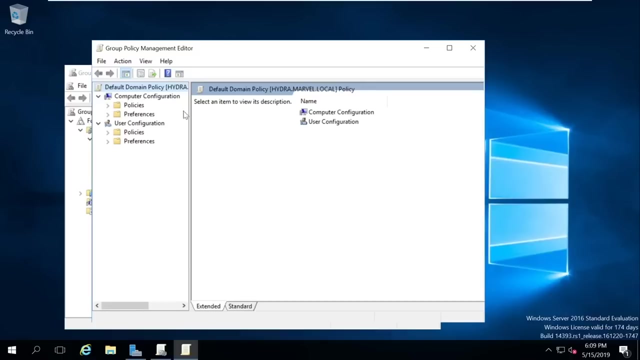 Okay, let's click on that. Okay, Okay, Let's click on that. So from here, you're going to see default domain policy. we're going to right click on that and select edit. From here we're going to be under the computer configuration. 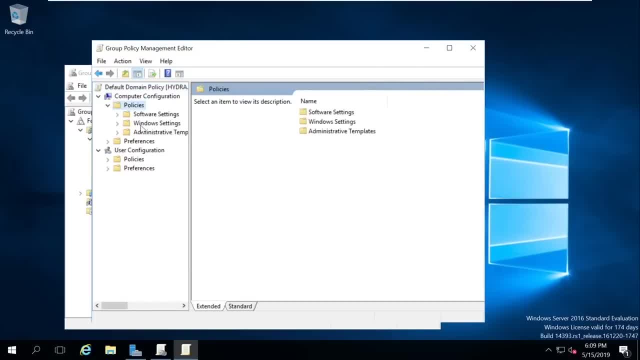 And we're going to say policies. Then we're going to click on Windows settings. We're going to come down near the bottom and select security settings- Okay, and then we are going to select local settings, Local policies- I apologize- right up here. 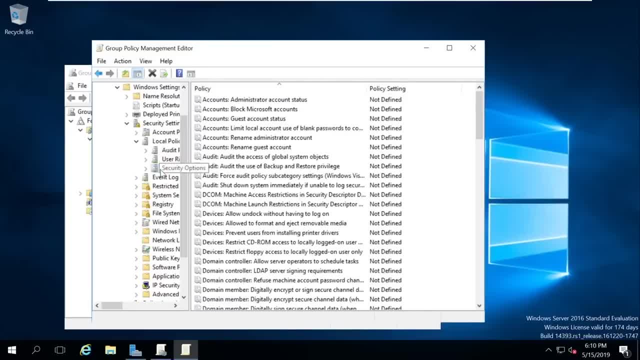 And then security options. So if you need that again we are in computer configuration policies, Windows settings, security options. Okay, Security settings, local policies, security options. Now you're going to scroll down until you see Microsoft client- network client actually. 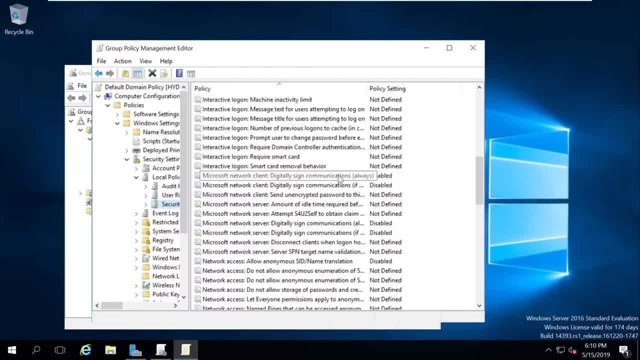 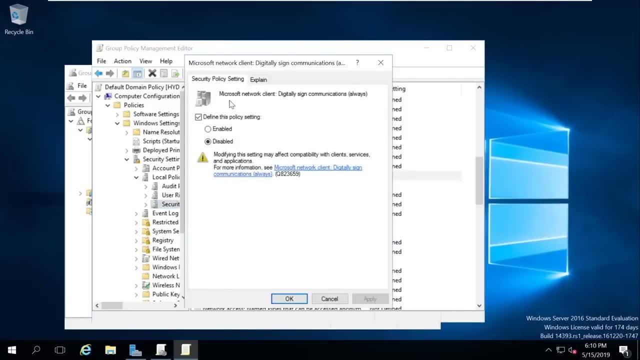 And you're going to see here it says digitally signed communications always And also if server agrees. I just disabled both of those. So you come into here and you say, hey, sign the communications. No, let's not do that. 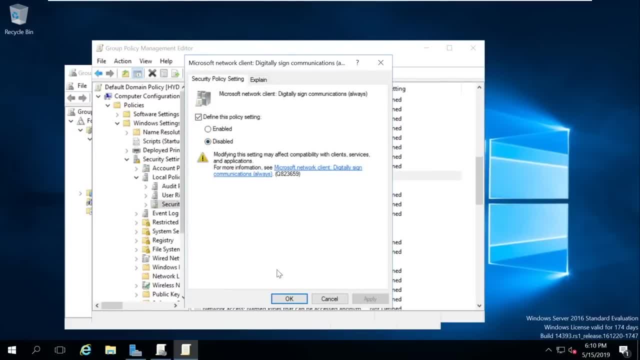 We're bad admins, right? So we're going to say disable And we're going to hit save And we're going to hit okay, We're going to also do the same for if the server agrees, just say disable defines policy. 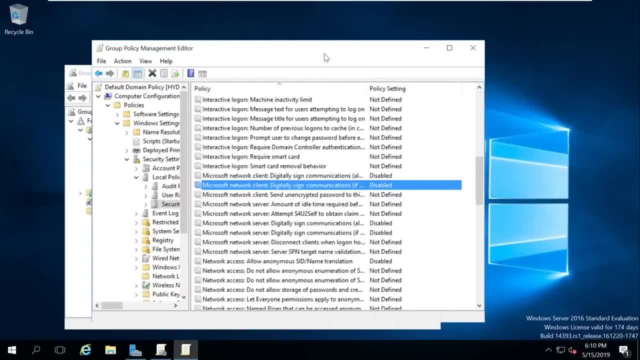 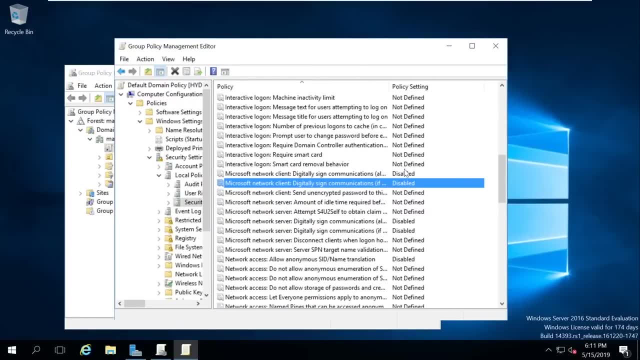 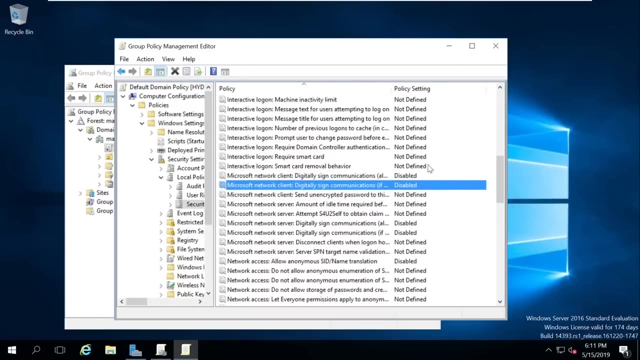 say: okay, You may need to reboot your your machines or do a GP update to actually push this policy By default. I believe it's actually off. I'm just enabling this here, But for for the purpose of keeping up with you guys, I'm just going to reboot both my. 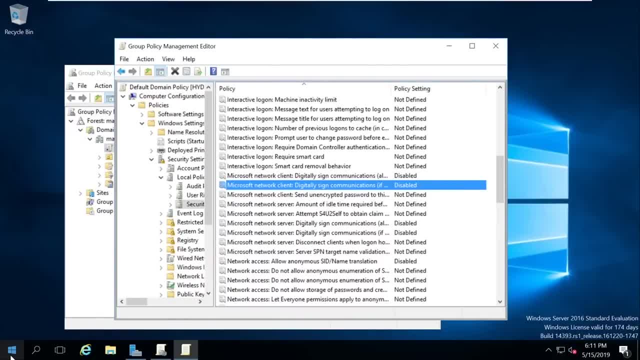 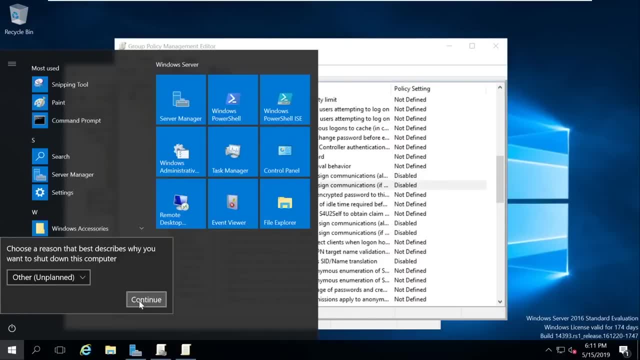 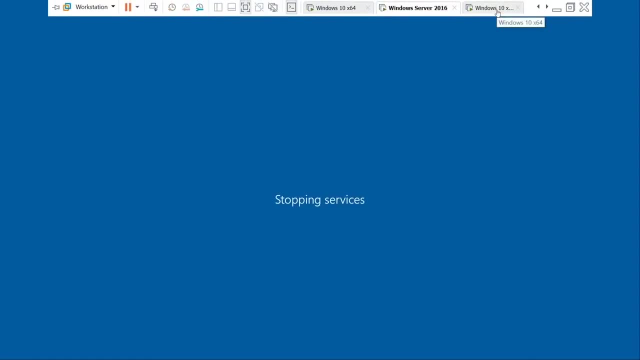 machine, my domain controller, um, and the machines that we need to complete the attacks. Let's go ahead and just reboot. Thanks guys, I am the best domain admin. We're going to reboot here as well. Make sure it picks up the policy. 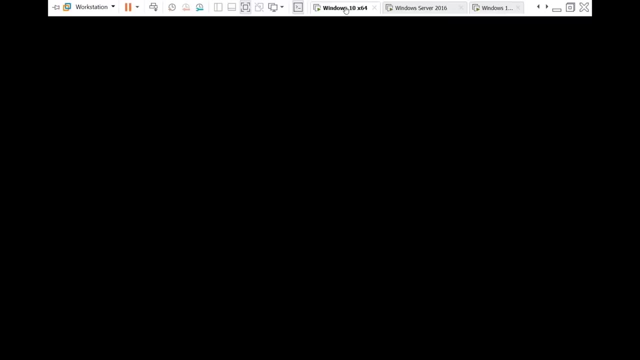 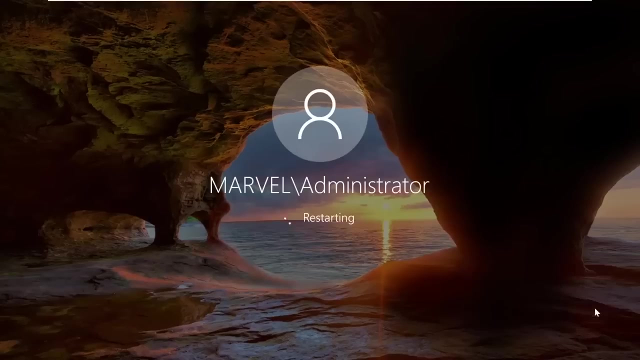 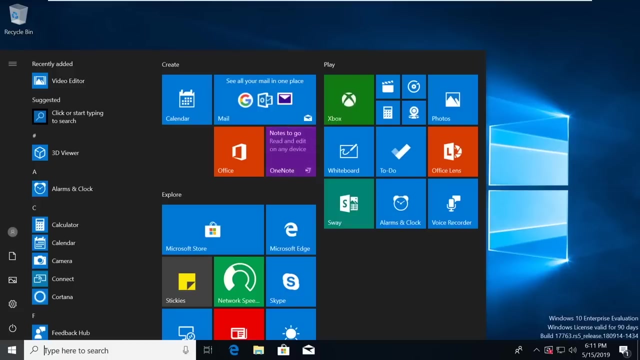 Oh, it wants us to update and restart Jerks, man, Jerks. Okay, Let's reboot here. All right, Before we reboot this machine, we've got a couple of things I'd like you to do, So what we're going to do is we're going to right click. 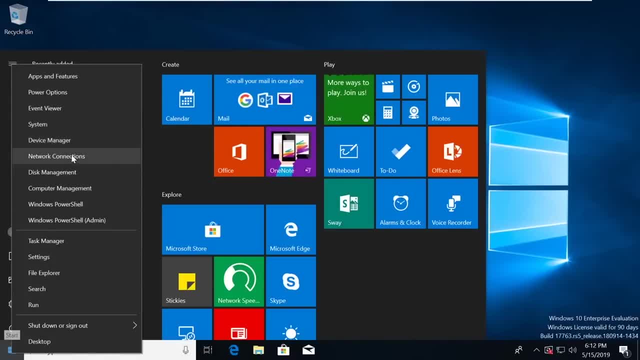 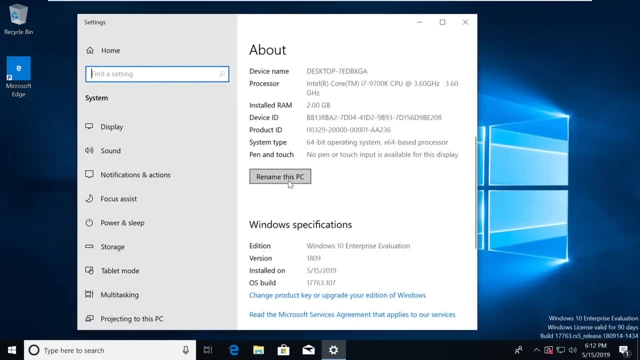 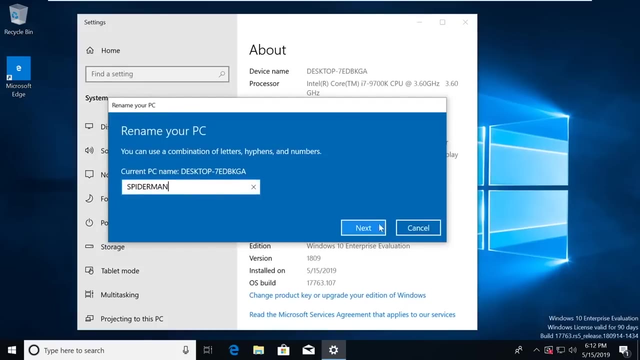 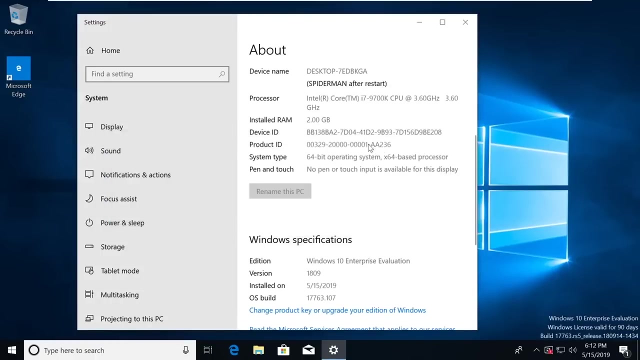 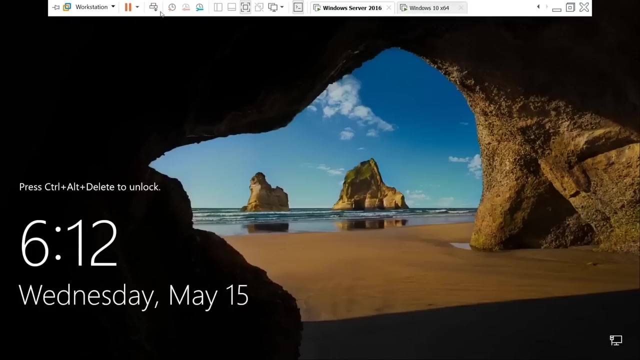 We're going to go into the uh system here. I like to rename the PC. What's up? Hey bro, We're going to name it Spider-Man because it is Spider-Man's computer. We'll restart later. We're also going to need to join the domain which. let me pull up these domain server real. 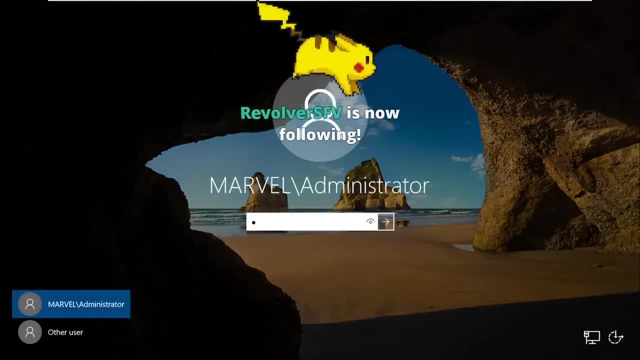 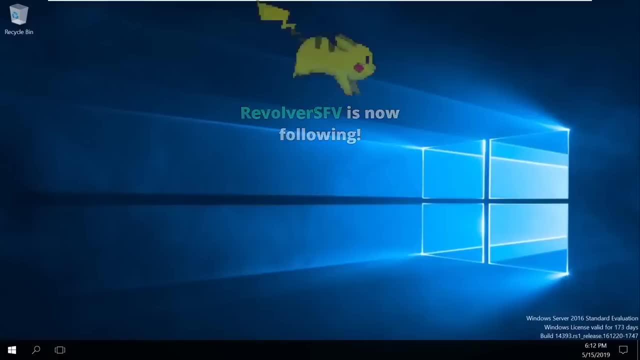 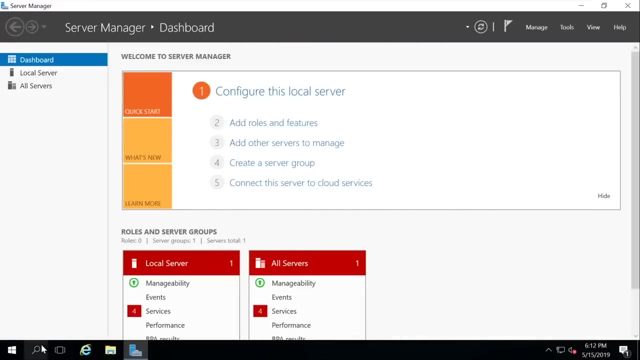 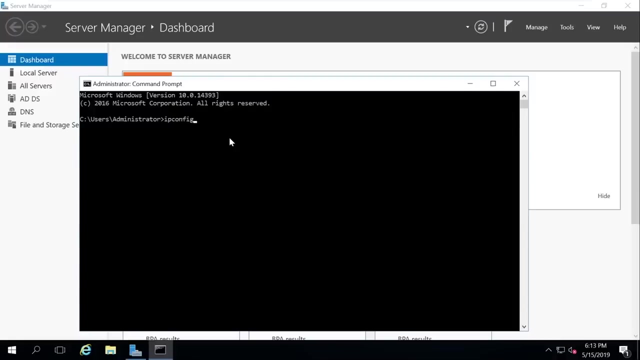 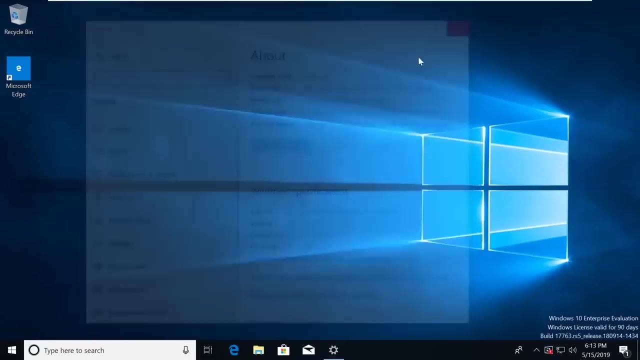 quick Login. Okay, Yeah, Thanks, And your username should be Tom Holland. I don't disagree with you. All right, let's pull the IP off the domain. Okay, It's running at one 37.. Okay, Okay, somebody did message me last week and tell me how to get to the network. 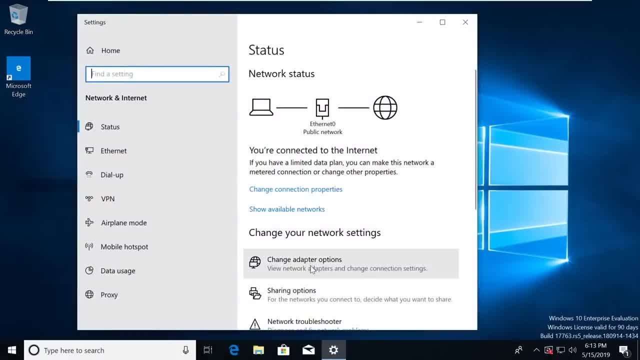 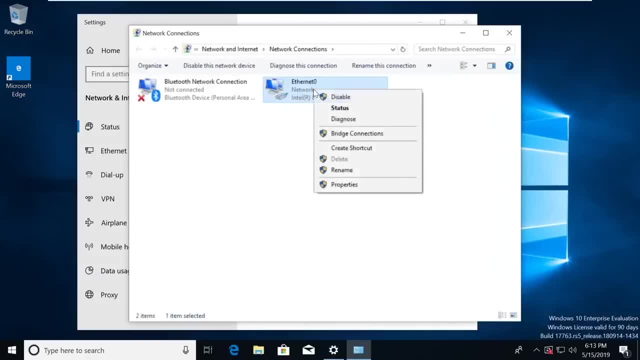 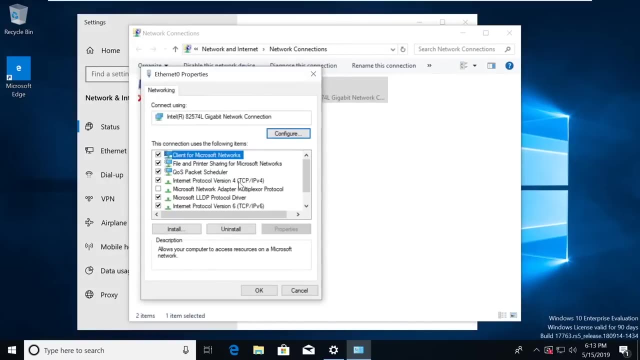 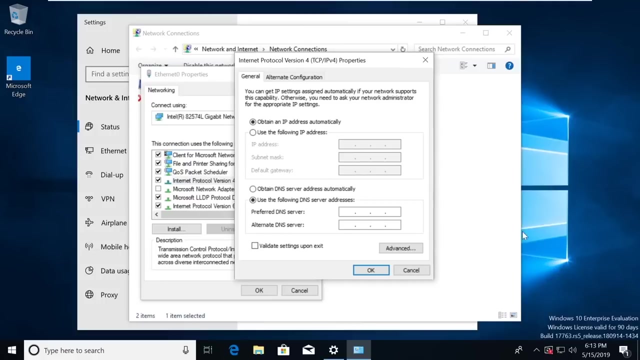 I still don't know. so I just type in network And there's change adapter options. here You're going to right-click on Ethernet 0, go to properties, Double-click on IPv4. And we're going to set DNS. So we are going to point it directly at our domain controller. 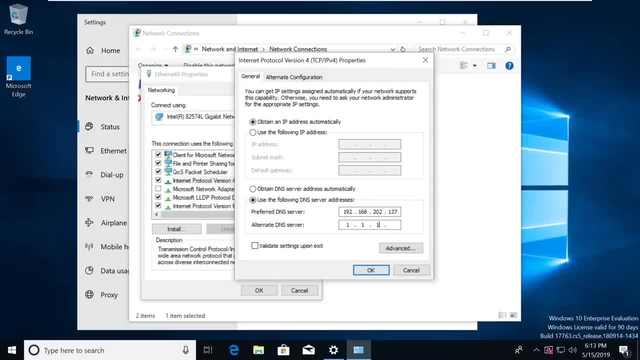 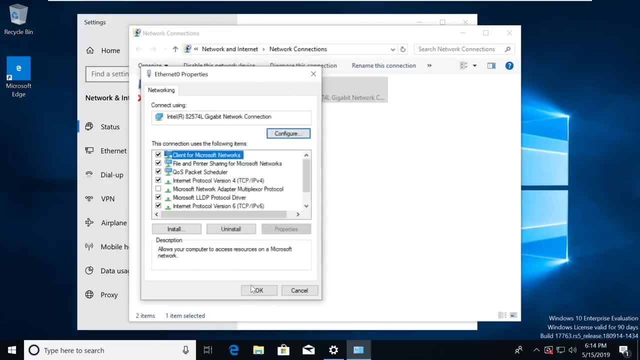 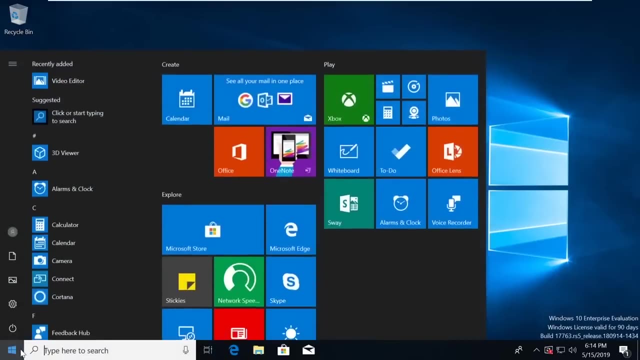 And since all of you homers wanted ones last time and I gave you eights, I'll give you ones this time. All right, Now that we've got our DNS set up, we're going to go ahead and set up our DNS. We're going to say domain. 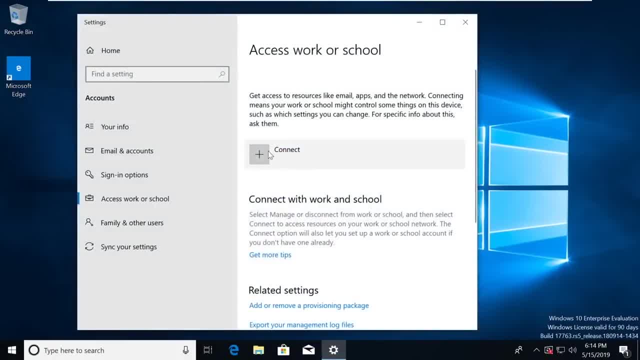 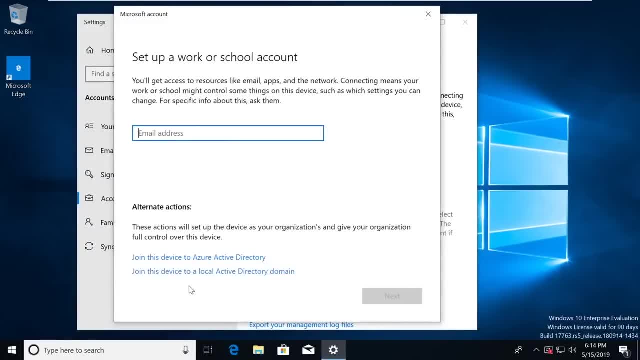 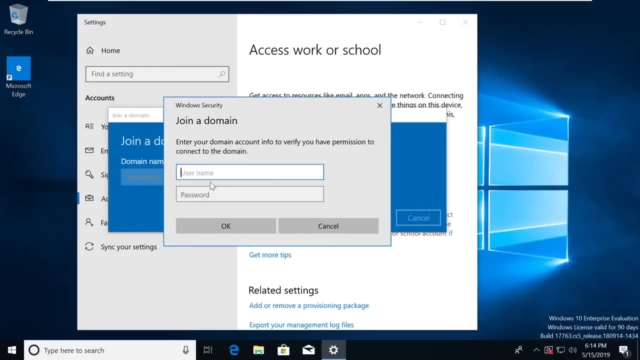 It's going to say access worker school. Click on that. Click connect, Set up a worker school account. We're going to actually say join this device to a local active directory. What's the domain name? Mine is marvellocal, Okay. 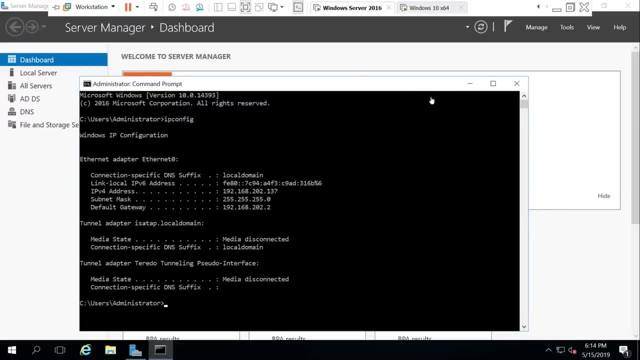 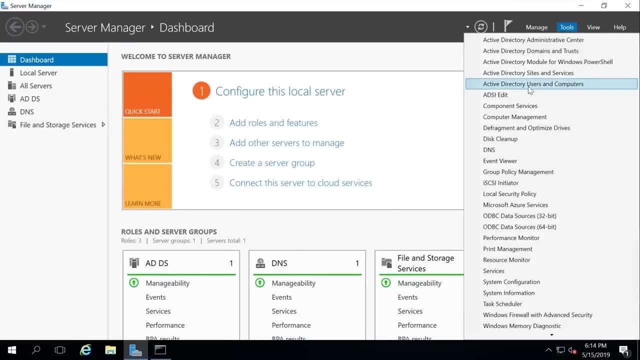 And oh, I forgot, I don't have an account for good old Peter here, So let's go into the server We're going to. We're going to go to tools, active directory, users and computers. Go to users. 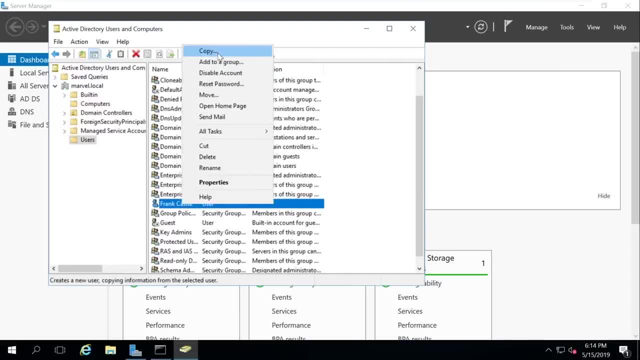 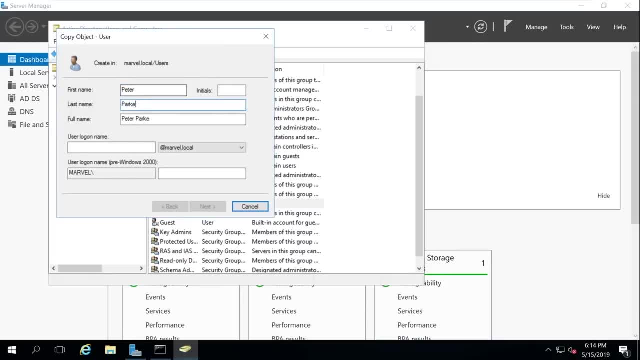 I'm going to right-click on Frank Castle and just say copy. We're going to take all of his policies. We're just going to call this guy Peter Parker. P Parker, first, initial, last name and cpacpl. 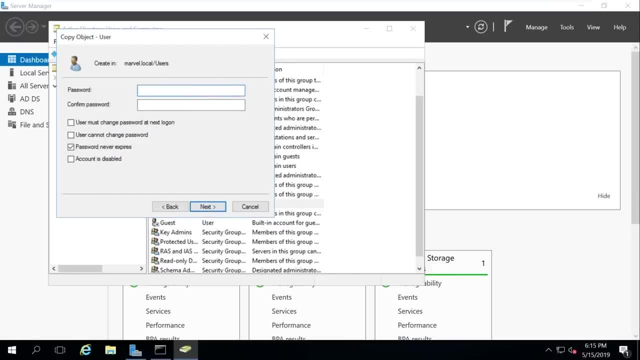 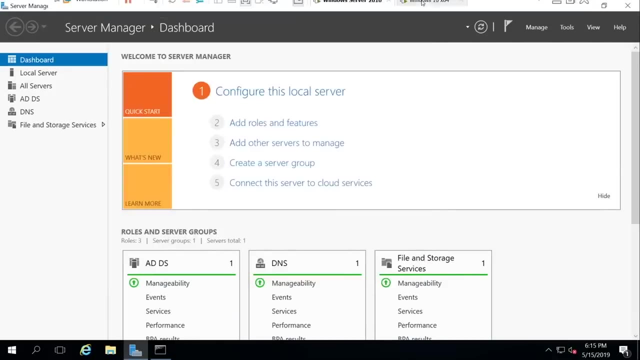 Thank you. I'll never remember that, but I thank you. Password never expires. We're going to make Peter have the password of password two Finish. Okay, We've got Peter there. now Let's go back here. P Parker. 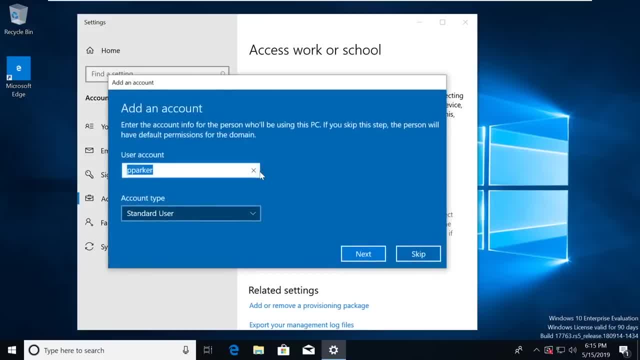 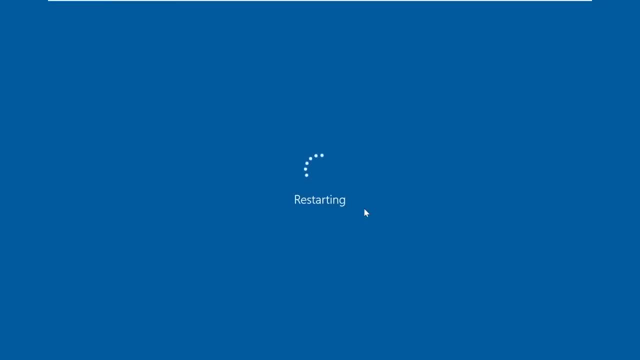 Password two, Standard account Next, And we're going to go ahead and reboot this computer, Of course. of course, we're hit with Windows updates, so let's take this as an opportunity to chat with each other about how awesome Windows is. 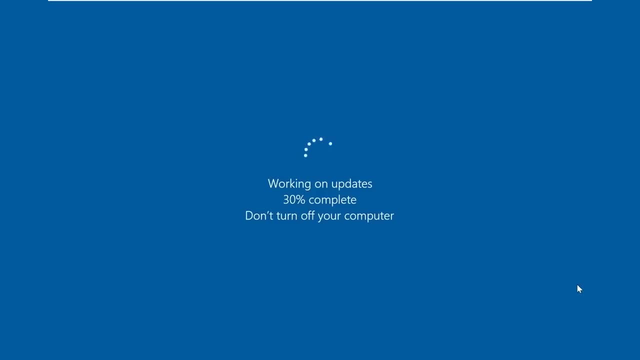 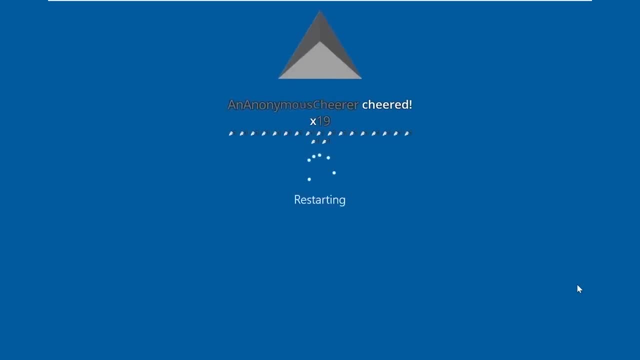 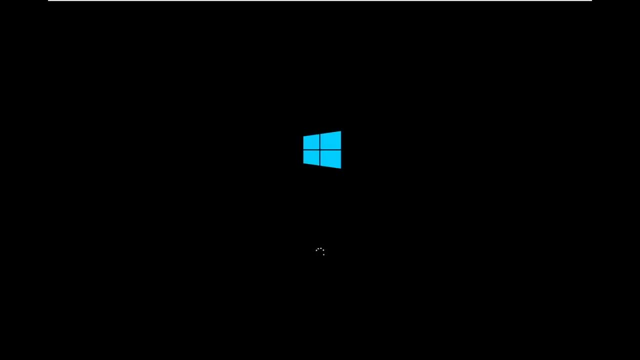 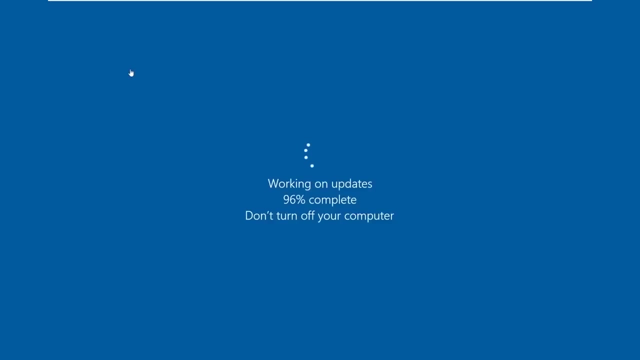 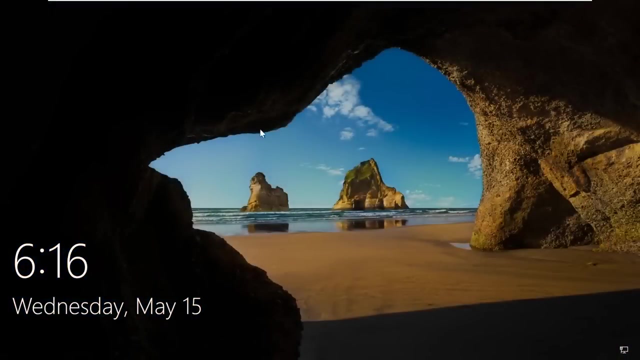 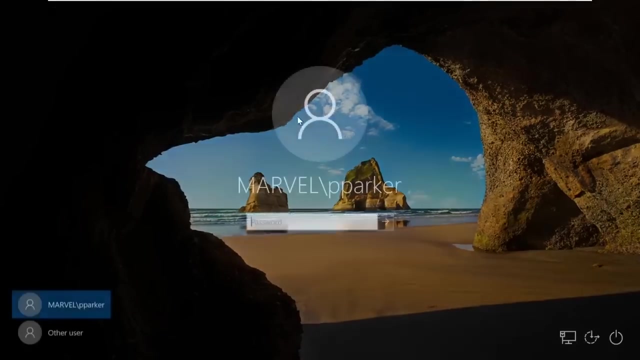 Will I do scammer streams in the future? I don't know what kind of streams I'm going to do in the future. if I'm being honest with you, I don't know where to go from here. All right, we're going to log in as Mr Parker. 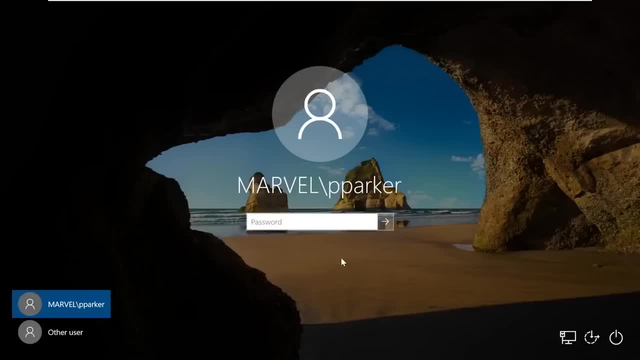 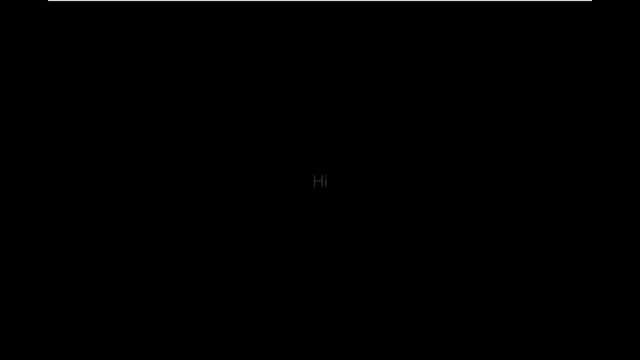 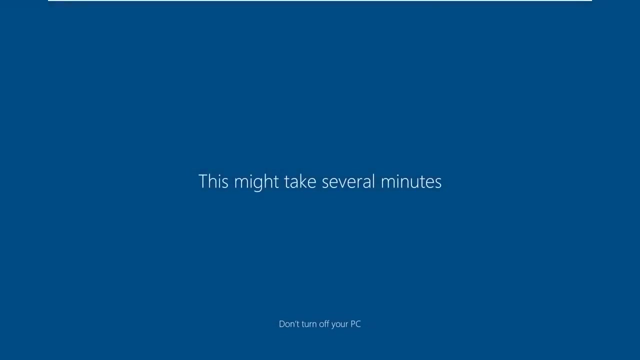 Actually, let's, let's log in as the. let's just make it easy and log in as the domain administrator. We're going to speed things up a little bit. Actually, I forgot to put Marvel in front of that. It's going to take just a second. If I'm ahead of you guys, let me know. 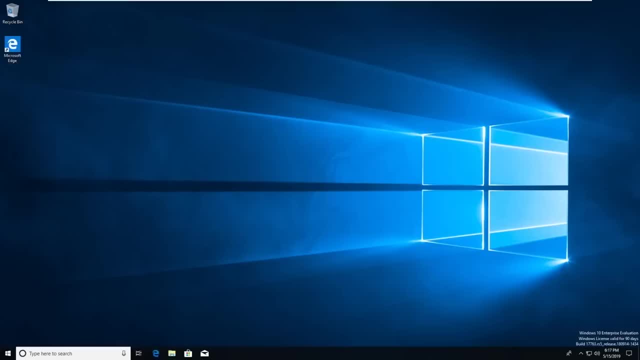 Okay, So we're going to have to make for this situation. What we're going to do is we're going to make this a little bit easier. We're going to make this a little bit easier. So we're going to make this a little bit easier. We're going to make this a little bit easier. 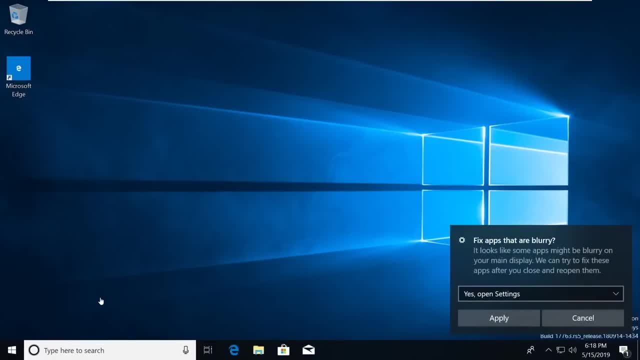 make Frank Castle an administrator. we're going to pretend that the account that we're relaying is an administrator or at least has access to this machine. Now, you see that a lot of the times where improper configuration, where a user has access. I have this in a recent internal pen test. 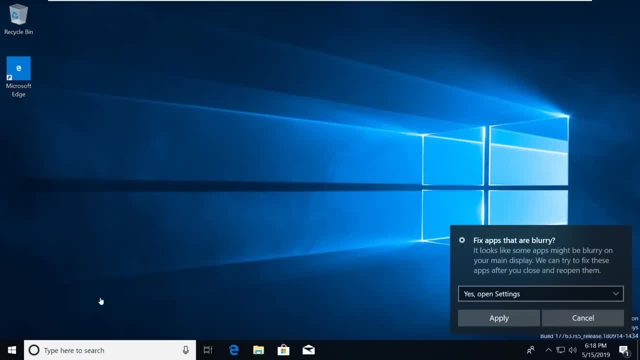 I cracked a user password and the user happened to have access to, you know, just one server. it was just one server, but that server allowed me to navigate to the domain controller. So you want as limited access as you can and least privilege, right? So what we're going to do? 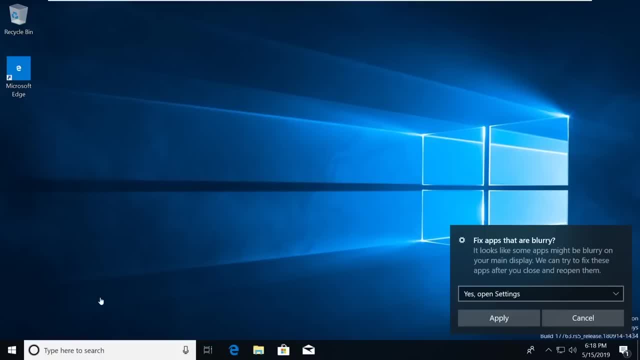 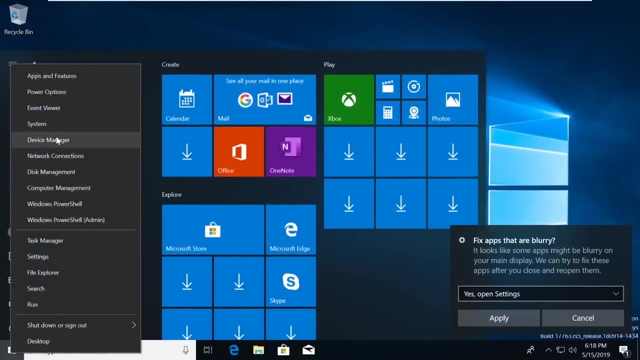 though, is we're going to demonstrate an environment where they're allowing their users to have some administrative privileges on multiple machines, And that's how we're going to be able to do this relay here. So let's go ahead and right click on this. we're going to go into 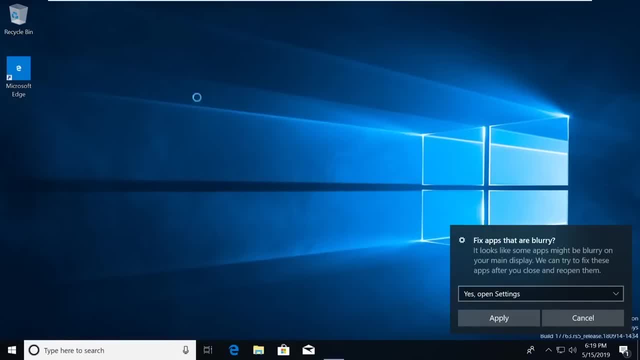 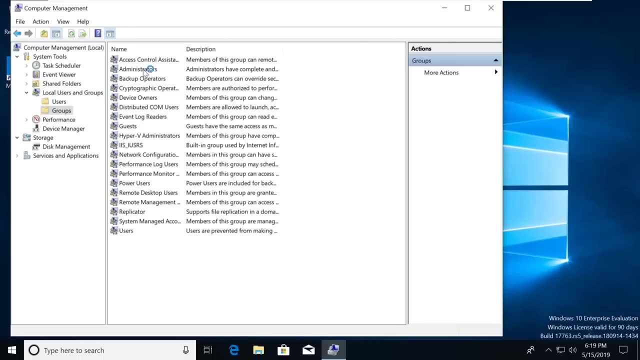 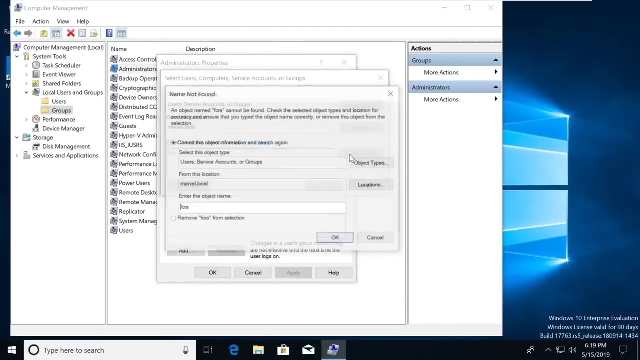 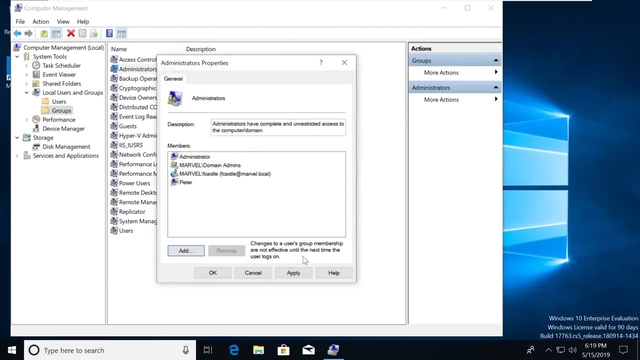 computer management again And we're going to go into local users and groups. we're going to click on groups again, double click administrators And we're going to add an administrator here of Frank Castle, If I can spell it Okay and apply that. 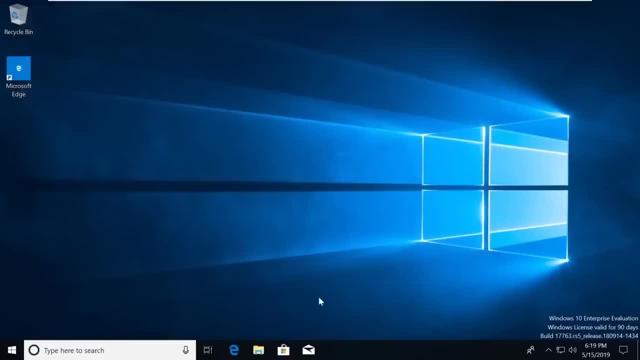 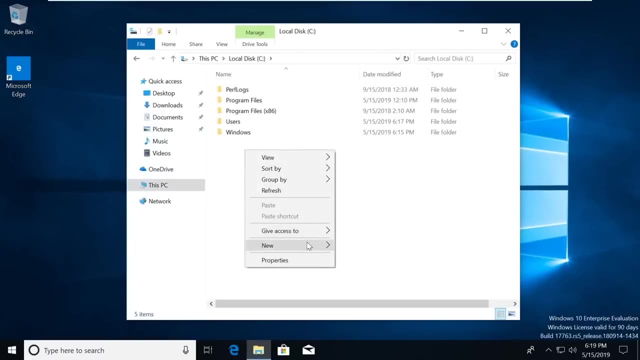 So now he's part of the local admins. We're going to come in, we're going to go to this PC, we're going to go to the C drive, we're going to right click and we're going to create a new folder, going to call it scans. 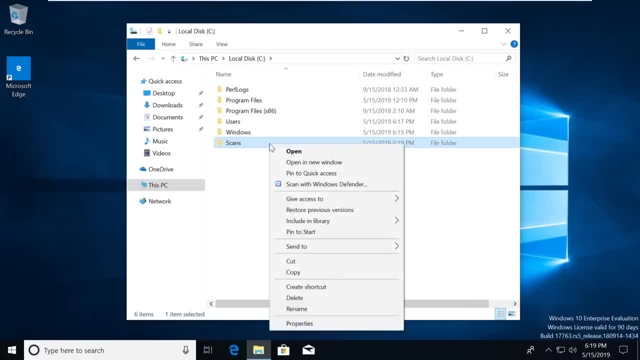 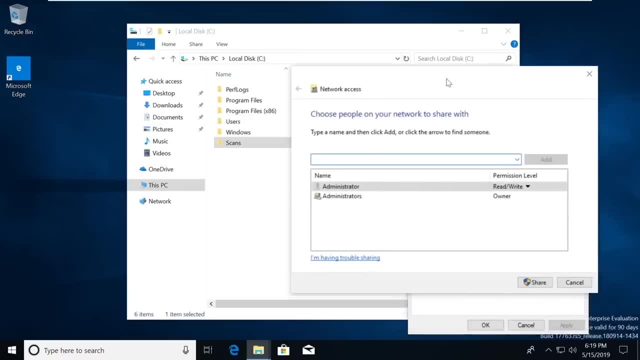 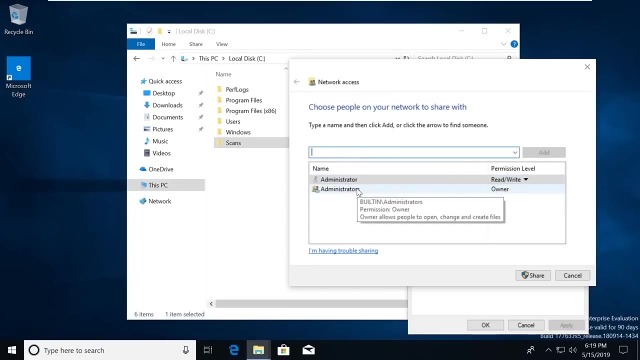 Same thing, no different. Going to right click on that. go to properties Sharing. we're going to share this sucker. OK, we've got administrators. have read write administrators built in, have ownership. Just to make sure we're not missing anything, we're going to go into whoever's coming in and we're going to go to Biden. certain, we're going to go Yoda. 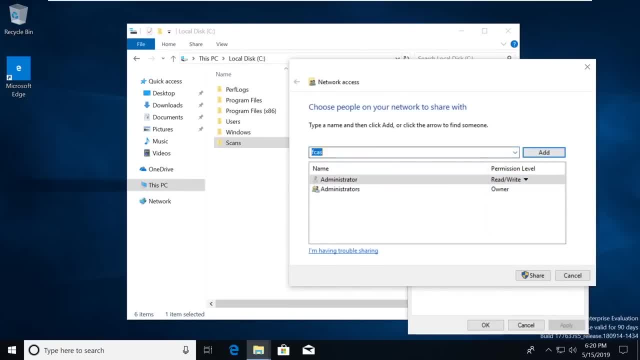 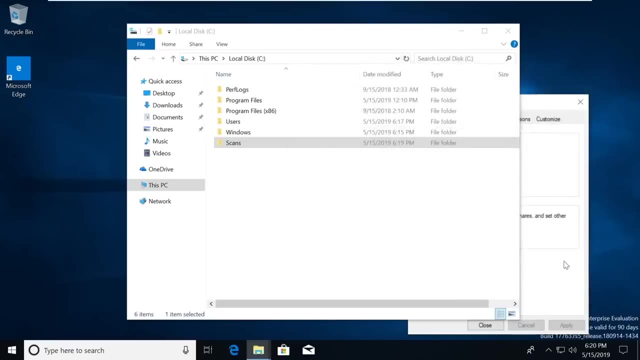 Just to make sure we're not missing anything. Just to make sure we're not missing anything, gonna give F Castle his own as well and we're gonna give him full read write and we're gonna share that. So now this is sharing. we should have SMB open on the. 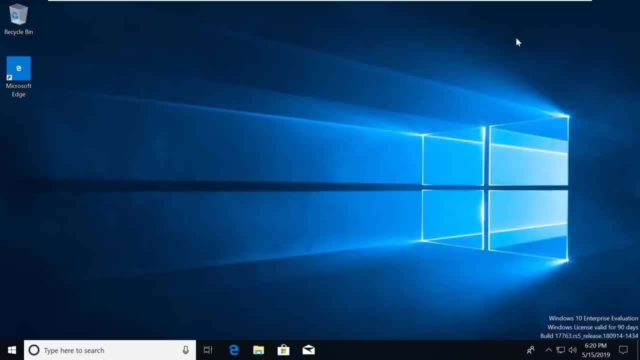 machine. Do I often see domain admin user accounts separated from IT staff? No, I have seen that one time. It made it a lot more difficult to exploit the environment, but we still ended up doing it. However, they were doing a great job with that. We were able to capture their- like you know, their base IT accounts, but 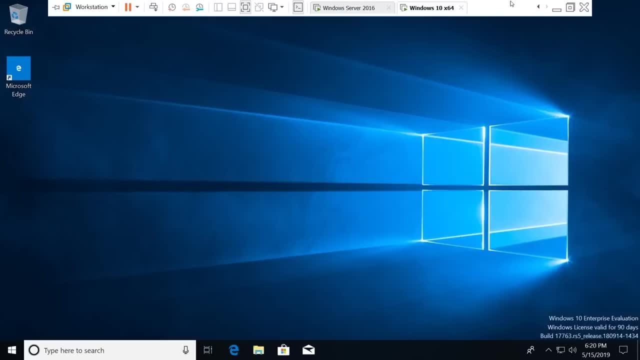 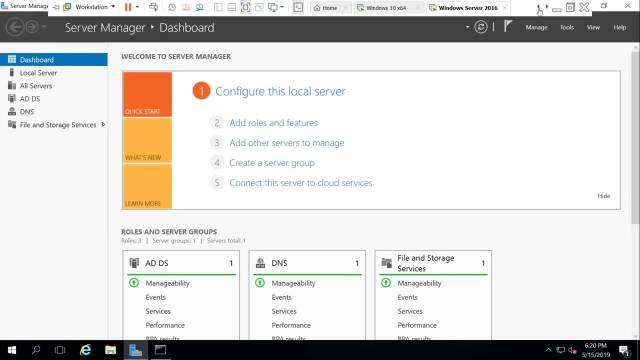 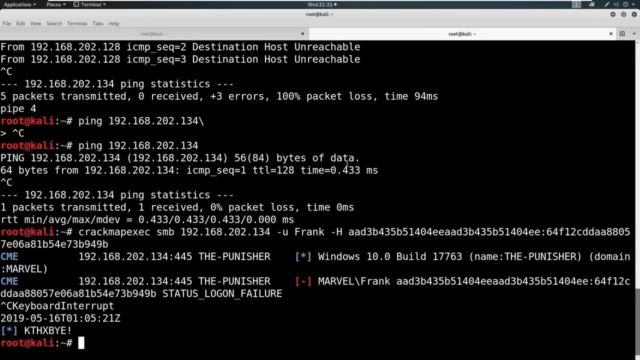 their domain admin accounts had really really long password policy and it was. it was fantastic To actually see an environment like that, but you don't see that a lot. All right, we're gonna go to Kali now and we're going to find responder again. I think it's in users share responder. 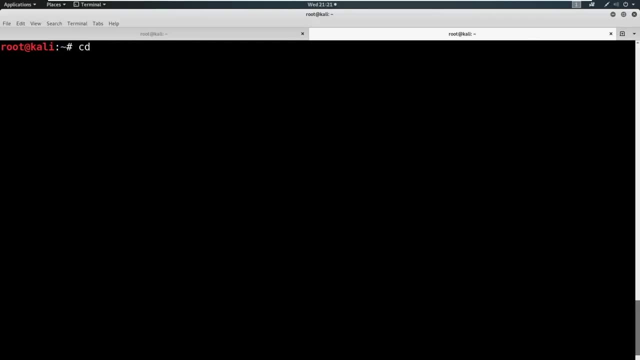 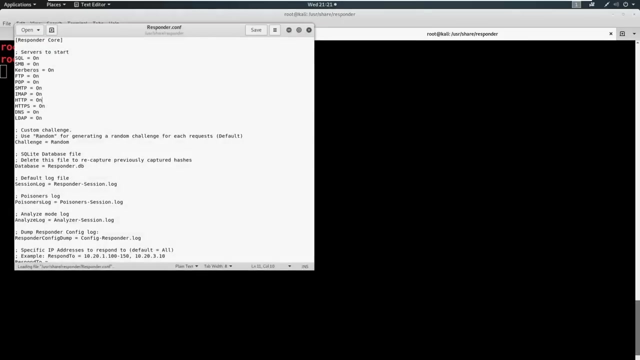 actually, yeah, so mine is in user share responder. Okay, and we need to make an edit here. Okay, and we need to make an edit here. Okay, and we need to make an edit here. So what we're gonna do is we're going to gedit responderconf, We're gonna edit. 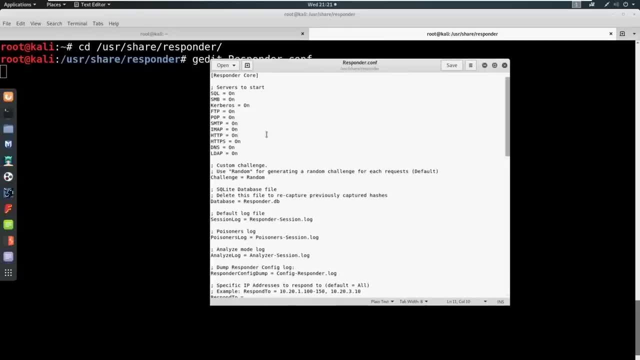 the configuration here. We need to turn a couple things off. We're not going to be starting an SMB server, nor are we going to be starting an HTTP server. So make sure again: SMB, oops, SMB is off and HTTP is set to off. Okay, we're gonna save that. 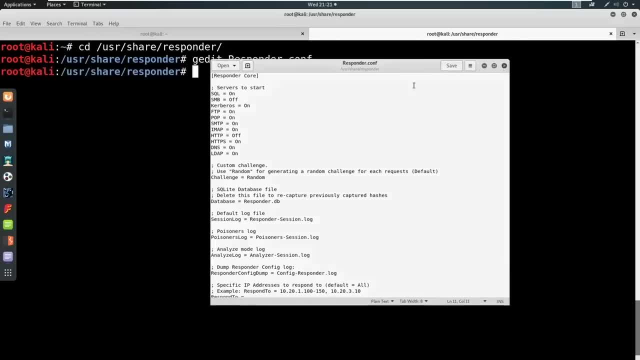 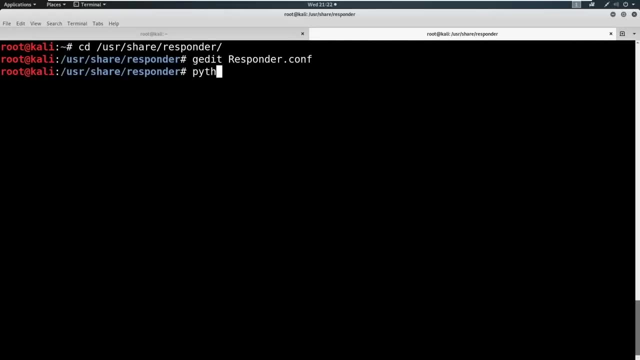 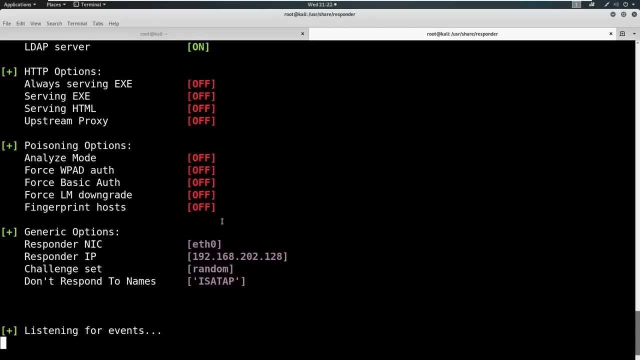 Now we're gonna fire up responder and that looks something like Python responderpy, and then we say "-i eth0-rdw". Okay, the firewall should not need to be off for PSExec. Okay, the firewall should not need to be off for PSExec. 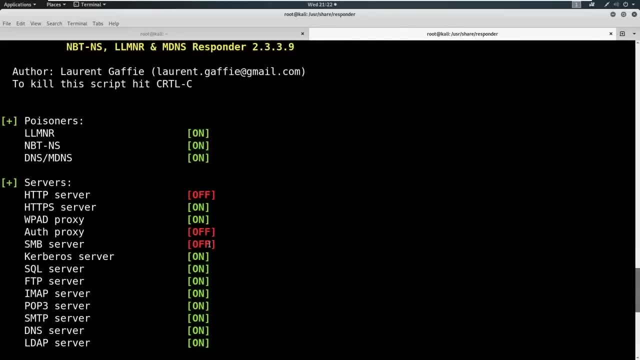 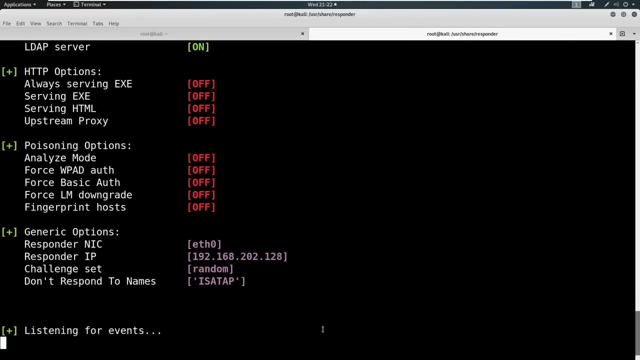 So okay, here we are. Now let's talk about the situation again. We've got the HTTP server off. We've got the SMB server off. We are sitting here listening for events to happen. Okay, when a hash comes through, like it did last time, we're going to use another tool called NTLM relay X and we're going to use that to relay the NTLM hash. We never have to crack this hash. We're going to take the hash, pass it to a 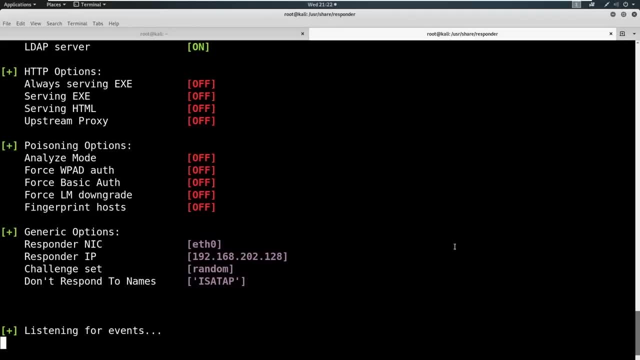 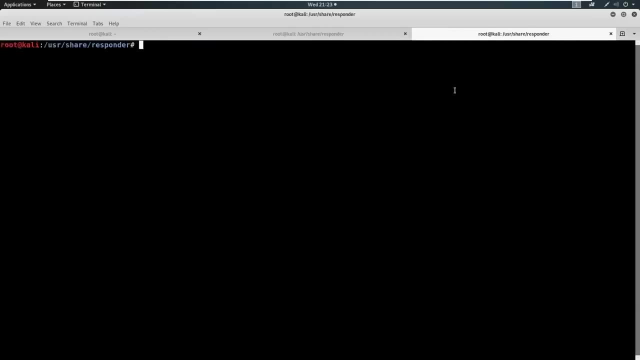 an SMB and try to gain access that way. This is where SMB signing is important. If you have SMB signing disabled- which it is in most environments- this is a killer right. So what we're gonna do here is we're gonna create a new tab and we're 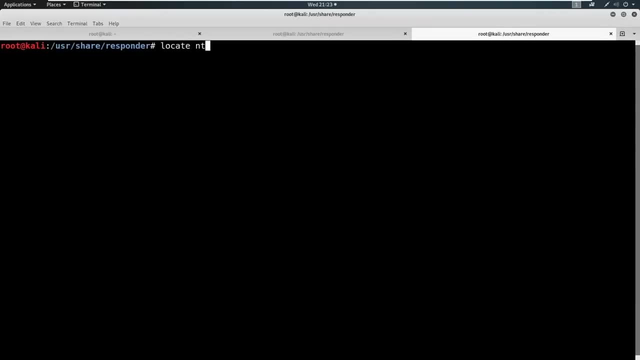 gonna say locate and we're just gonna find I don't know where it's at. it's gonna be in a different folder: NTLM, relay, Xpy. Okay, it's gonna be in the impact folder. So we're gonna say cd opt, impact it examples. Okay, now we're gonna fire up. 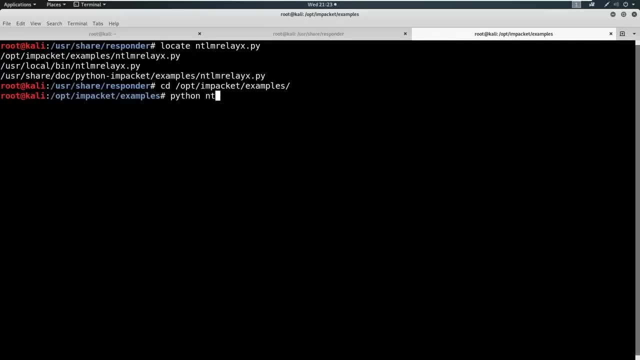 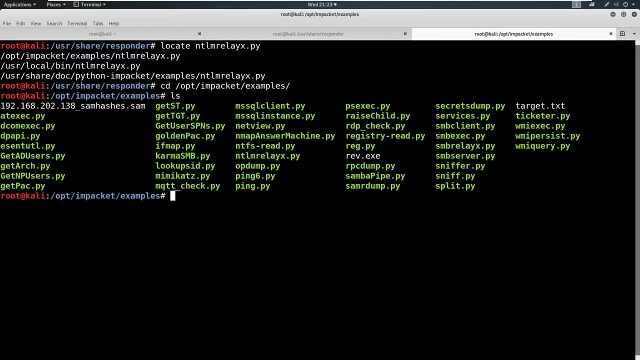 NTLM relay. They say Python, NTLM relay, Xpy. Actually I got ahead of myself. We have a target that we need to specify in a text file here. So if we ls, I've got a target dot text. If we go in here and we just say cat, target dot text, it is 138. I. 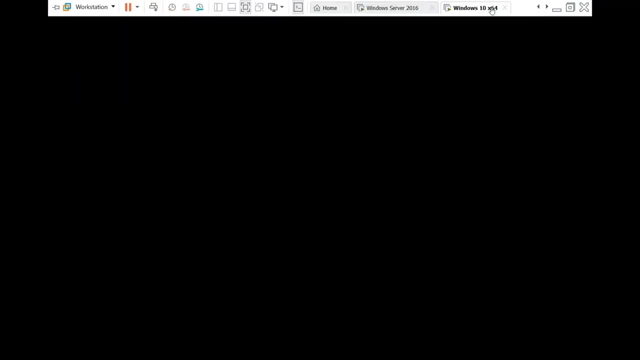 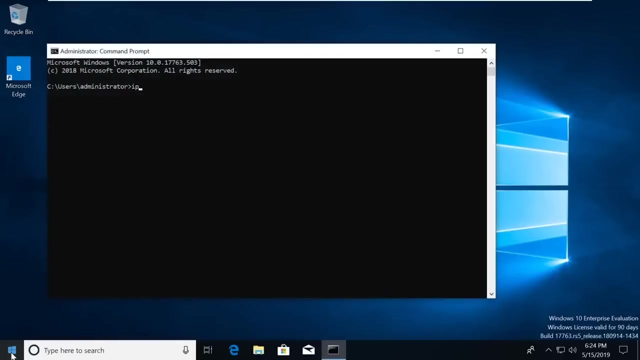 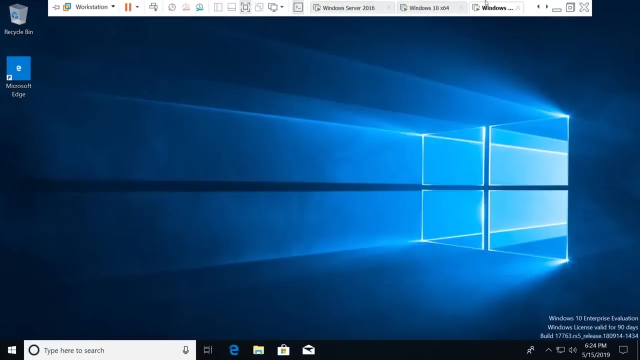 don't know if it's 138, but we're gonna have to make a file for it. So give me one second. So we say: command IP config. It is 138 still, So make sure you have a file with your address for the machine of Peter Parker. 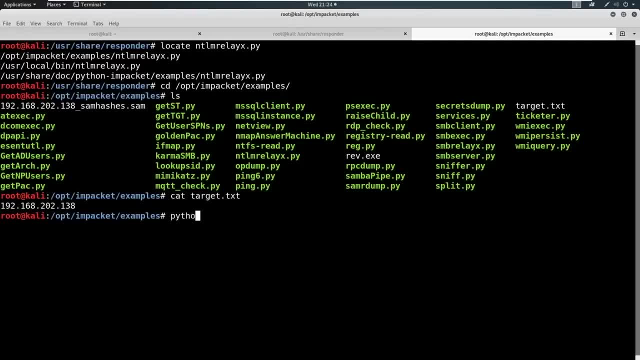 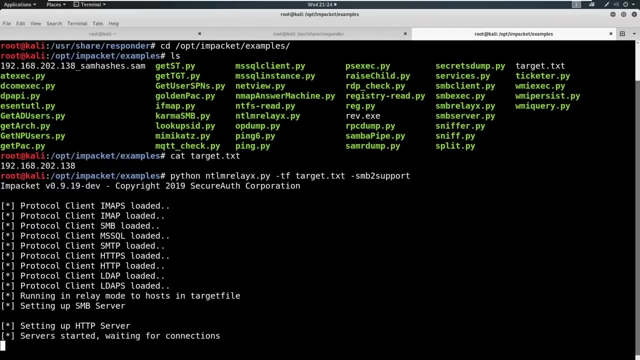 Okay, one second, one second, one second, Yeah, and we're gonna use this document: PolymerPy. OK, We're gonna say okay. So we're gonna say: Python, NTLM, relay, Xpy, dash, TF, target dot text I like to put in SMB to support: fire that guy. Now, that guy is. 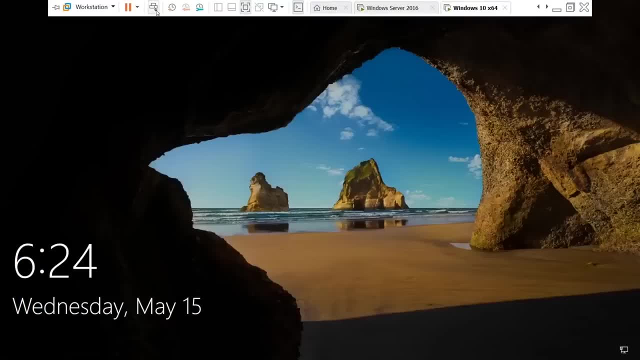 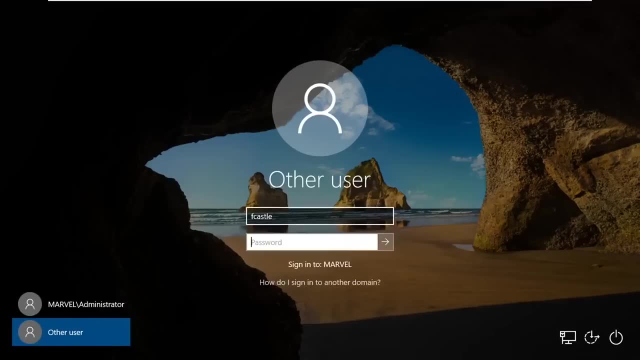 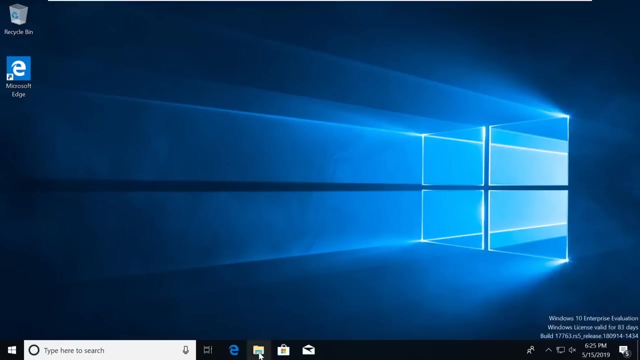 gonna sit there, Listen for the NTLM relay and then it's gonna relay it to the machine that you're choosing in, as actually Frank to Frank's machine, and pray that this works. Live demonstrations are always the hardest. Says he can't get to the. the hack me. 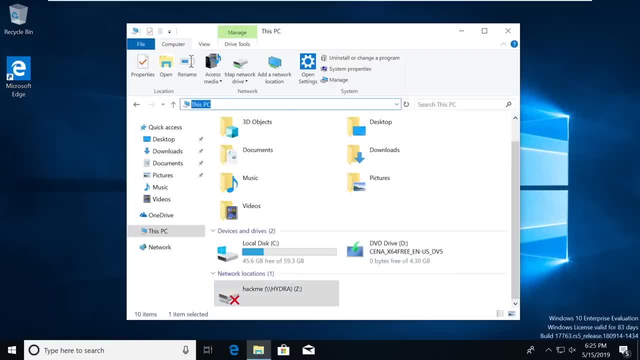 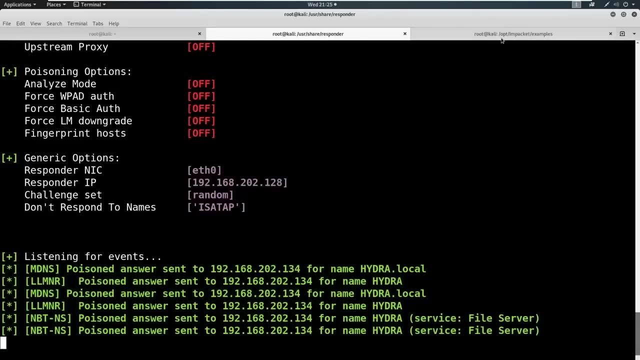 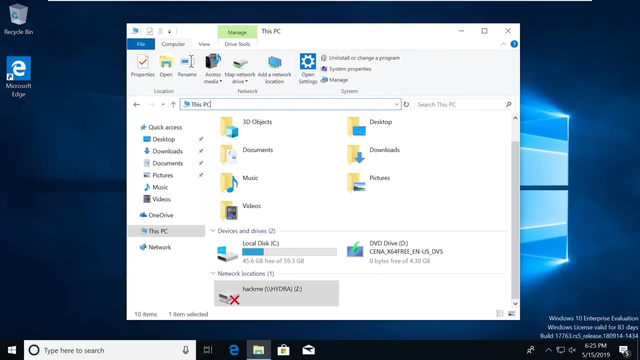 that's not good. Actually, I wonder if that DNS issue just caused it to relay. It did not. There was poison. Okay, let's try. let's try just pointing it. So point it towards your attacker machine. Let's go back to Cali, wherever. 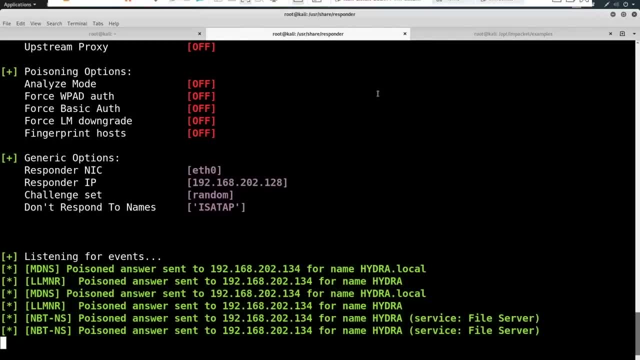 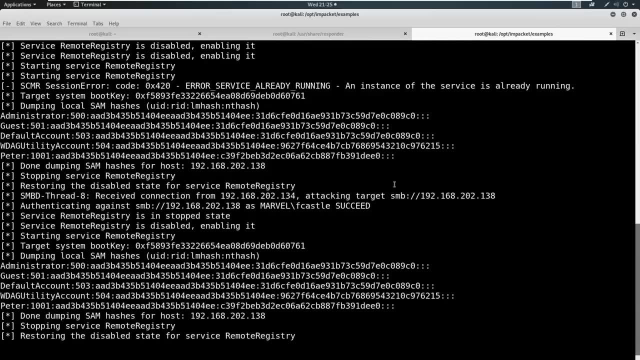 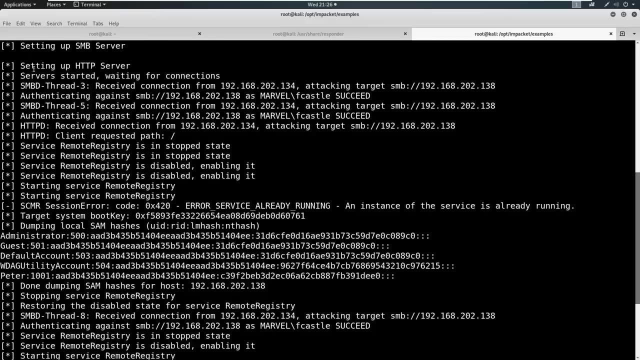 that is, Am I not on 128?? Oh wait, it happened. It did happen actually in the the initial Okay, so we did relay, We did relay. So if you come in here, it takes the connection from 134 and it attacks 138.. You can see? 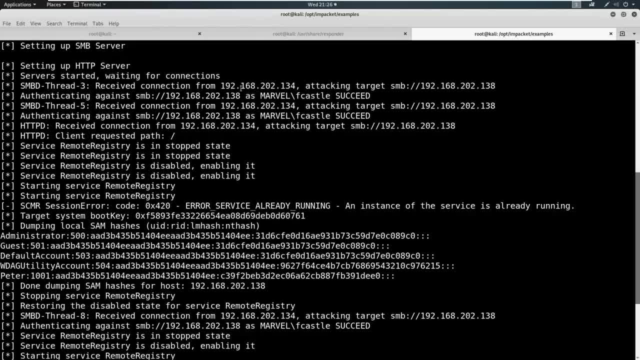 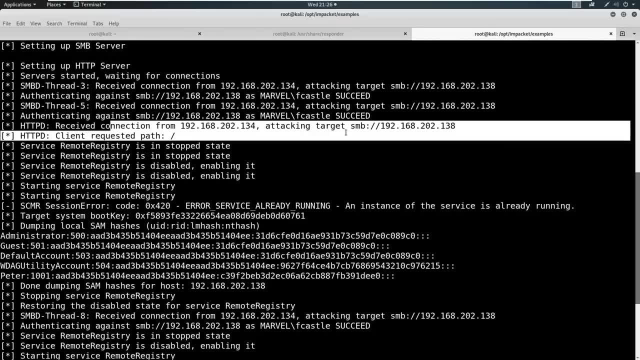 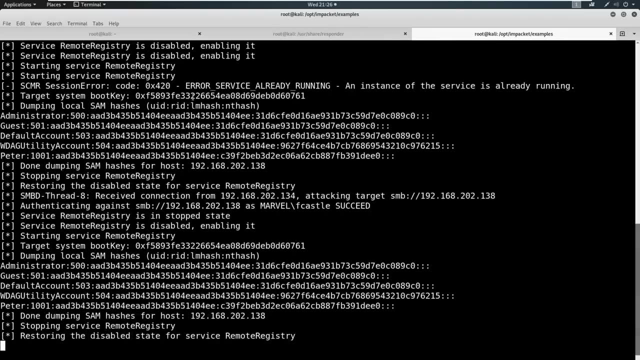 that Marvel F Castle succeeded with authentication. F Castle had access to 138.. Now, automatically it comes in here and it says: what can we do? Well, it's going to dump the local SAM hashes. Now we have the SAM hash for administrator and for Peter, So we're. 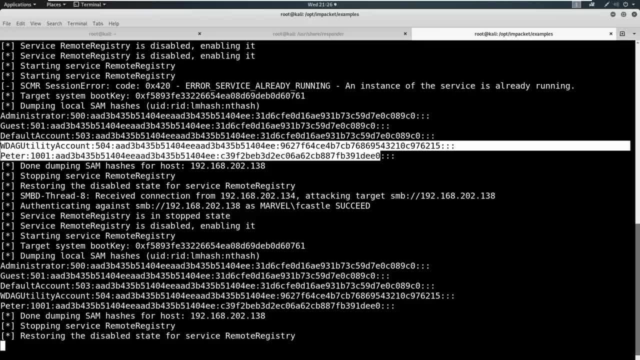 going to go in and we're going to try to log in with this hash on the computer to gain access. We're also going to try to pass these hashes around to see what we can do. We're going to try to take this offline and crack it if we have to. to. 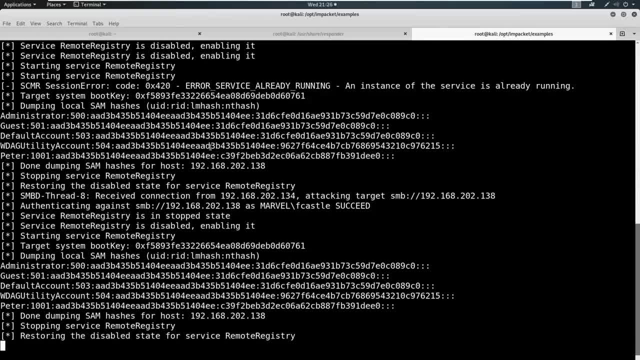 gain access to the machine. Now this is an example of NTLM relay, My challenge to you- and I said I was going to challenge you to do something- You can take this further. You can actually get a full shell from this, doing something called SMB relay. Same concept, just a. 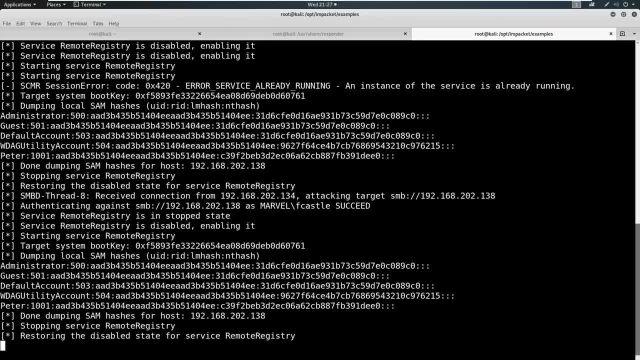 different, little bit different tool set. So that is my challenge to you: if you're doing this lab and you have successfully relayed, Now take it and see if you can get a shell. You're going to have to do some googling, figure things out, try a. 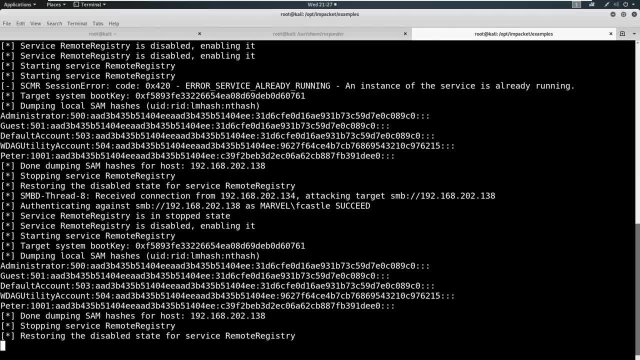 little bit harder, Whatever the fun lingo is. But that's my challenge now is to try to get a shell off this, either with a meterpreter or with using Empire, and see how far you can get. But this is the proof of concept that we can actually 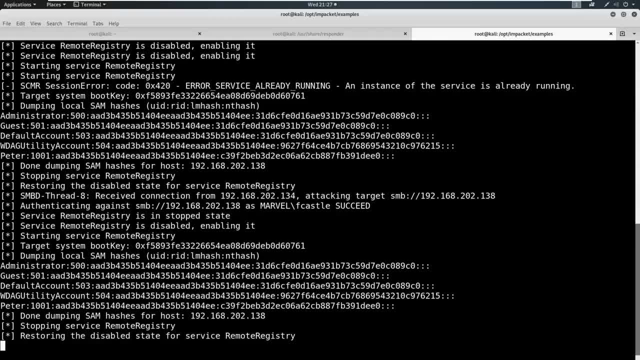 access the machine and dump the local SAM file. So very, very cool technique to use, Especially if you're not getting anywhere with the actual responder, The the password cracking. So Ruri's given out hints. He says Empire is the thing he uses for this. 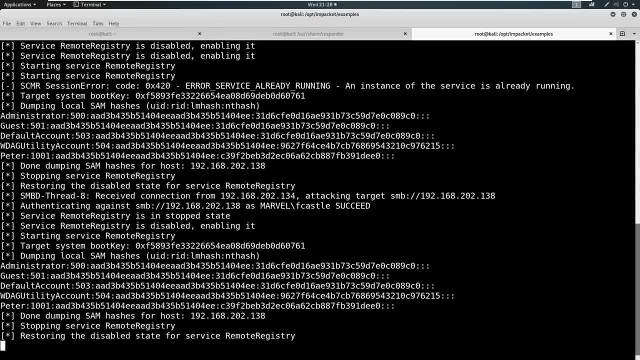 Yes, Empire is likely the way to go. If you look up most articles on how to do it, Empire is going to be in there. You may find one or two with a interpreter, but it does not hurt to learn Empire. So that is my challenge. That is it, And this lesson is officially over, right at. 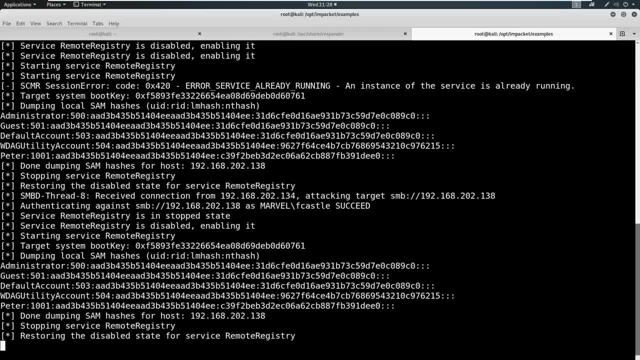 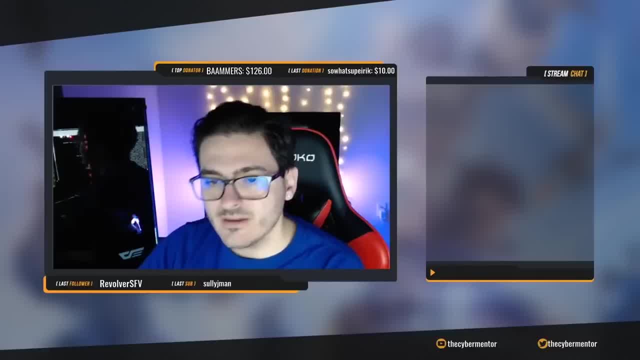 9.30.. So again, if you guys want to see round three of this, I am happy, happy, happy to do that. Please just upvote on active and upvote on blue. We'll do that. It'll probably be half of a. 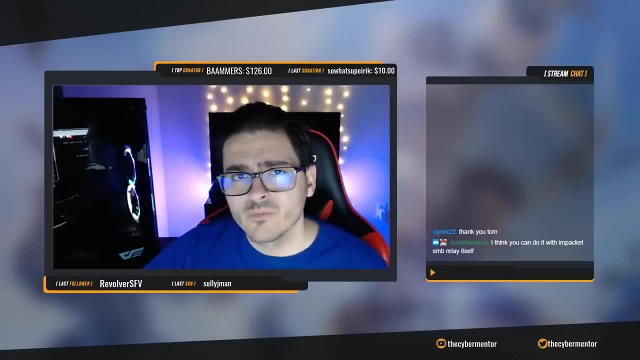 week, next week, And what we'll do, or half of a session, and then we'll dive into whatever, whatever we're missing. I don't remember what we're missing. We'll probably start into our pivoting lab, or we may cover the legal stuff and do a pivoting lab. 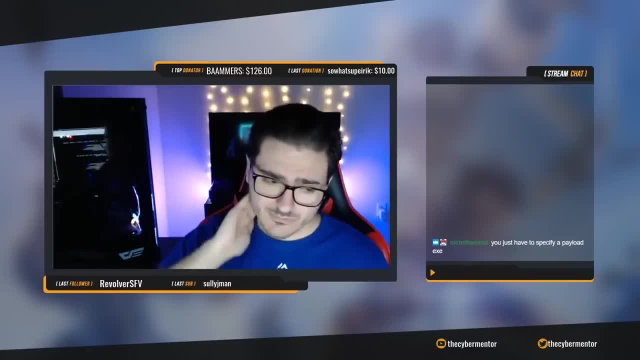 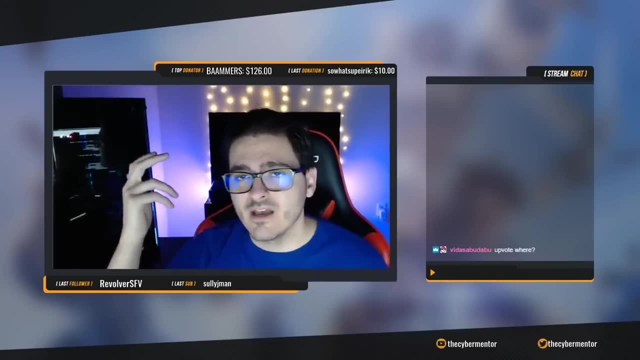 at the end I got to figure out how I want to do that. So I really do want to do a capstone. We'll see if we can do a capstone or we'll just do capstone lessons for a couple weeks after the. 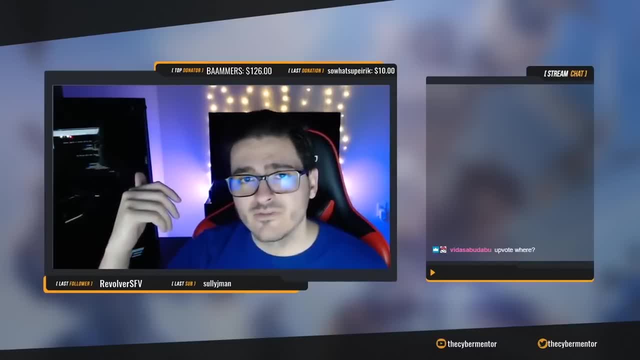 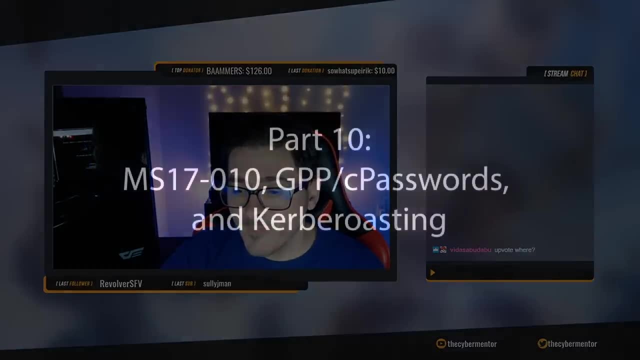 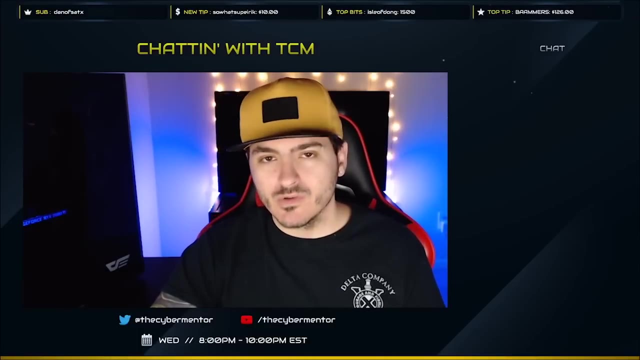 course ends, And that way you guys can get a feel for what my enumeration process is and how I really look through things. So that'll be fun. What's up everybody? So tonight we had some technical difficulties with Hack the Box. We're. 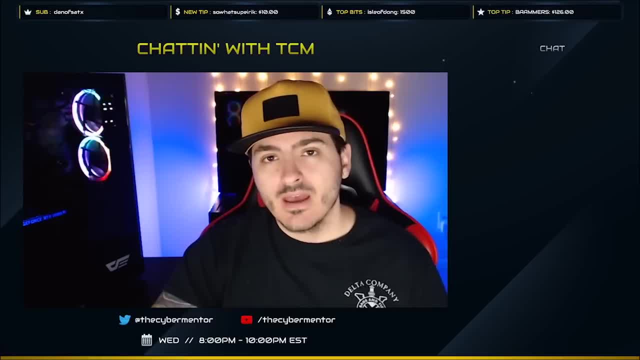 having some issues getting, you know, pings coming back and in connection to the boxes. When we did get connection to the boxes, we had just disconnects happening. We eventually had to change VPN connections a couple of times. So what you're going to see is a couple of hard. 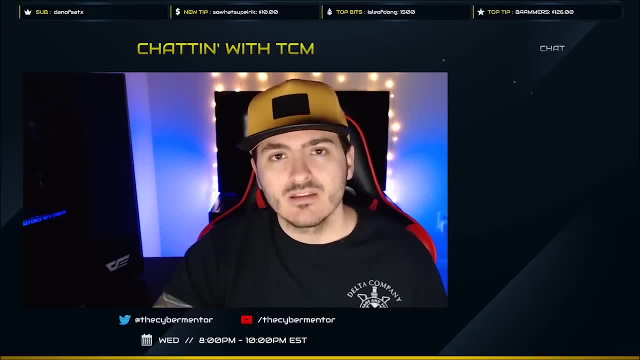 cuts in videos. I did my best tonight to edit the video down to where it made the most logical sense, And I'm going to show you how to do that. So I'm going to show you how to do that. So I'm going to. 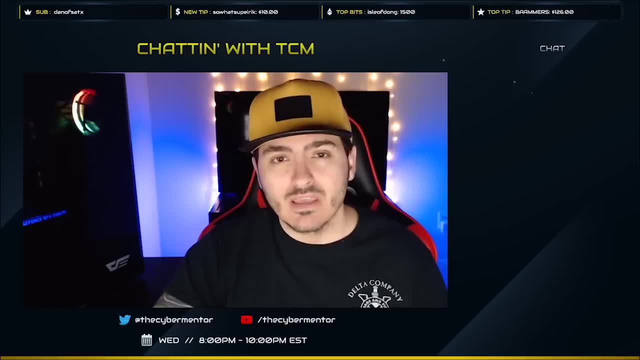 show you how to do that. So I'm going to show you how to do that as well as took out all of the technical difficulties that we encountered. So if you were a part of the live stream and you watched it live, thanks for sticking with me. You guys are awesome. If you're catching it on the 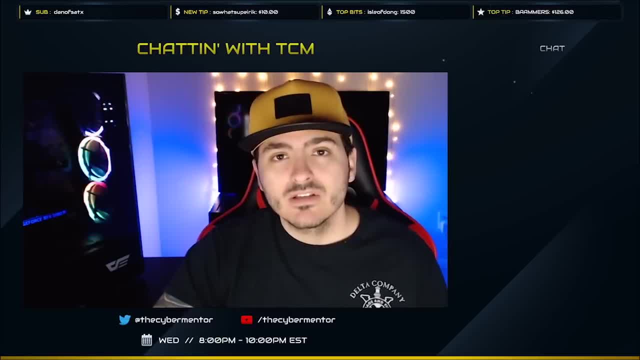 recording. hopefully I did a good enough job to patch things up and you don't really notice the difficulties. But if you do see some hard cuts, just understand that we were having a lot of issues getting connection to Hack the Box. So, without further ado, here is episode 10, part. 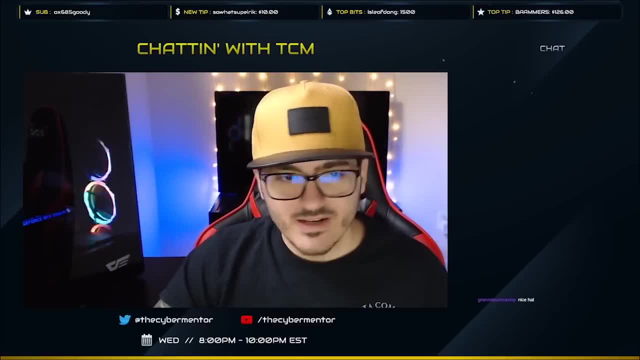 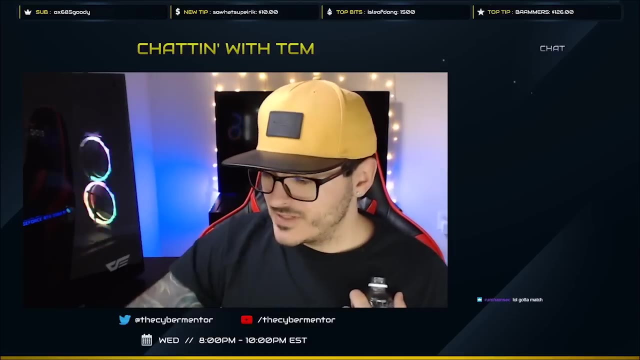 three of Active Directory Explanation. All right, it is 8.02.. I am done stalling. you guys Don't have a lot of PowerPoint. Got a whole three slides for you. Press my handy dandy new button, Boom, All right. So week 10, we are in the 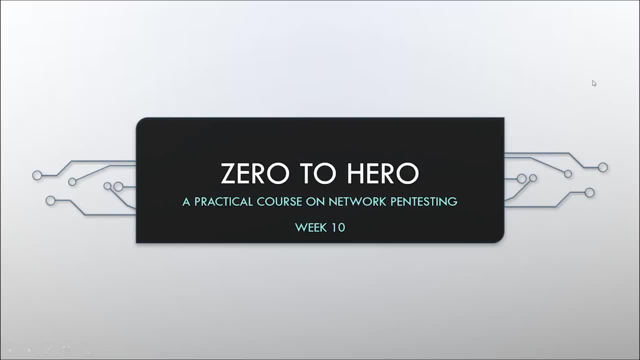 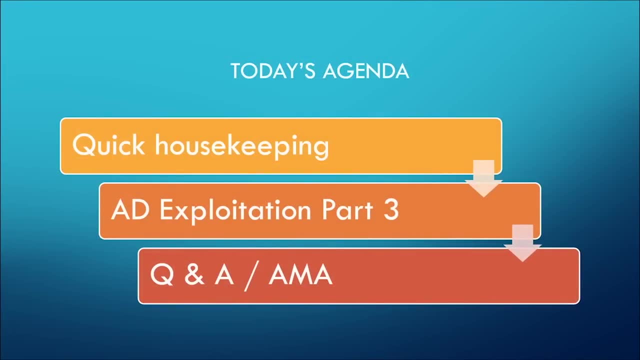 penultimate week. Next week is the last week, So we've got some quick housekeeping tonight, AD Exploitation, part three, and Q&A AMA. So I will talk about the AD Exploitation real quick because I didn't really put it into what we're doing on. 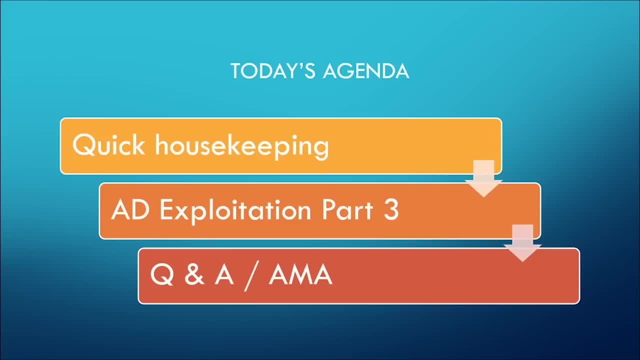 the housekeeping. We are going to be covering tonight MS-17010, very, very popular exploit. We're going to be talking about Kerberosting and we're also going to be talking about GPP and C passwords. So I'll also cover a little bit of Metasploit. We'll reinforce a lot of concepts. 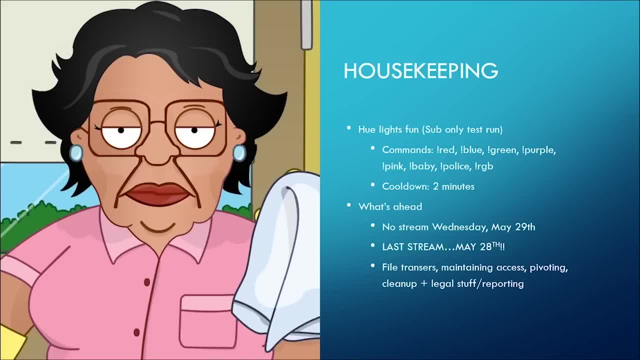 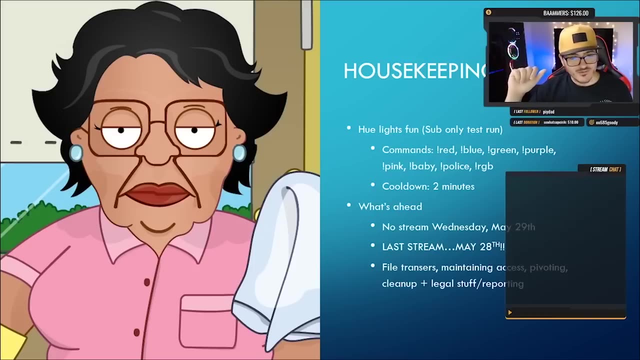 that you've seen the last couple of weeks and you're going to just see more of the mindset of what I would do in a real internal penetration test. So some housekeeping you saw behind me. Let me change the screen here. I have hue lights in the background. We're doing a test run- this: 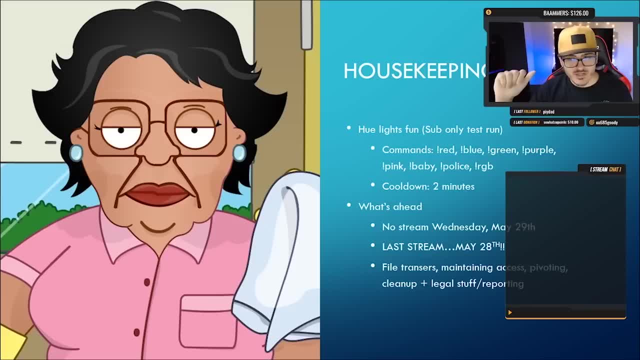 week subs only. If you are a subscriber, there are some special commands for you behind me that will allow you to change the color of my background. Now there is a two minute timer on it, but there is red, blue, green, purple, pink. baby is baby blue And you can see the police is going off in the 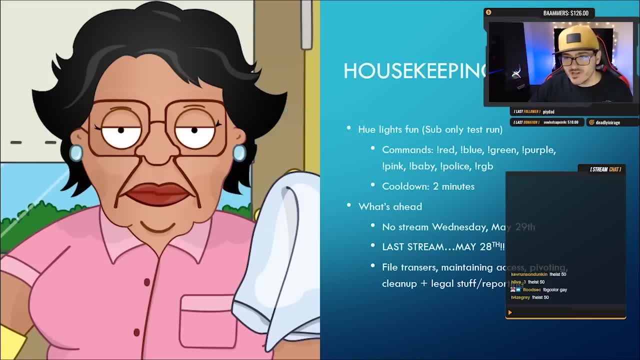 background for the subscriber, But you can also do the police and the RGB as well. So, thanks, Thanks deadly for the sub. I appreciate that. So yeah, keep that in mind If you guys want to play with the colors while I'm talking. 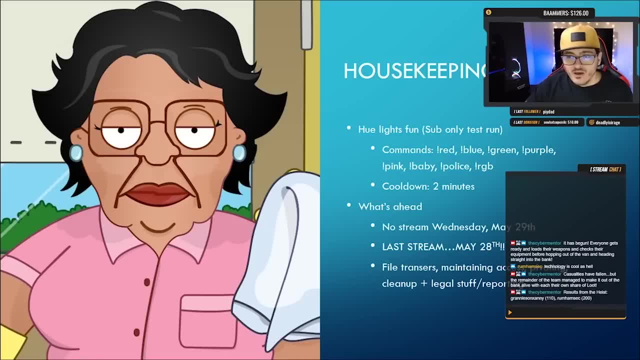 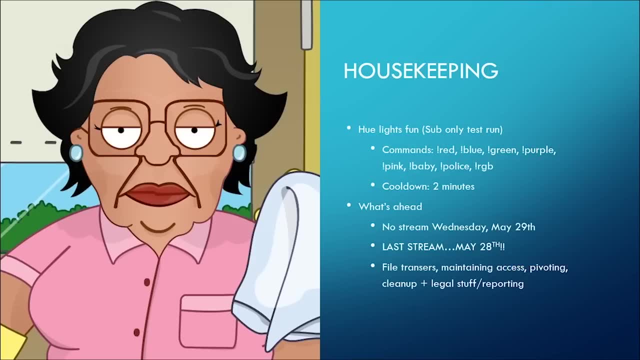 you're more than welcome to play the colors. Other than that, let me take this off. So there is no stream next Wednesday, May 29.. I will not be here Again. I will not be here. So last stream. the last stream is May 28.. We're going to be covering file transfers. 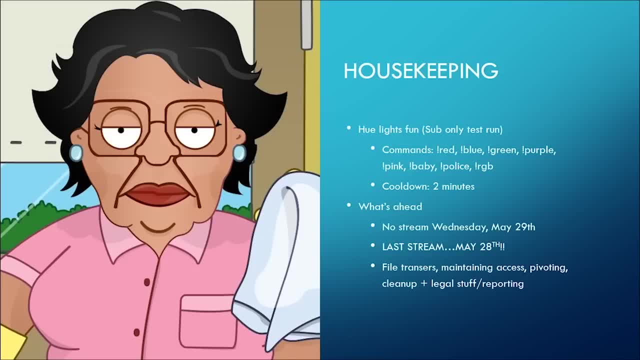 maintaining access, pivoting and cleanup. Second half of the night we're going to be talking about the boring stuff, which is legal documents you're gonna need to know about, And reporting will cover what a pen test report looks like and what. what are some good reasons for resources for building a pen test report? 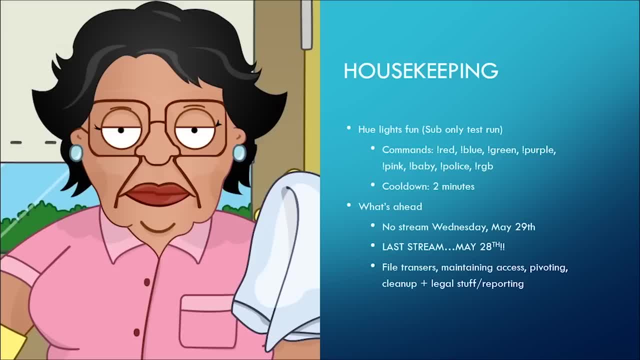 So the important stuff to know, Other than that tonight's lesson is going to take probably an hour. we don't have a lot on our plates, So just sit back and relax and enjoy this final 80 lesson And then we'll. we'll take it easy tonight And then next week. 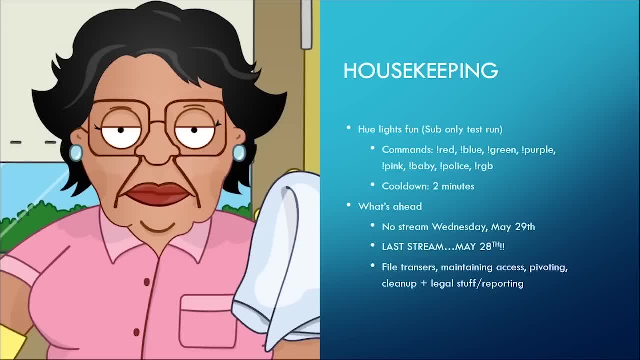 if you guys want to come up for something next week. I don't know what I'm thinking yet, But maybe we could do some kind of drinking game or something fun that we can talk about in the discord. But if you come up with something fun, I'll play along with you guys, Since it's the 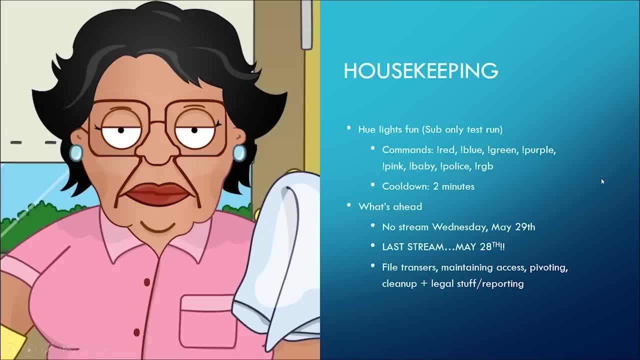 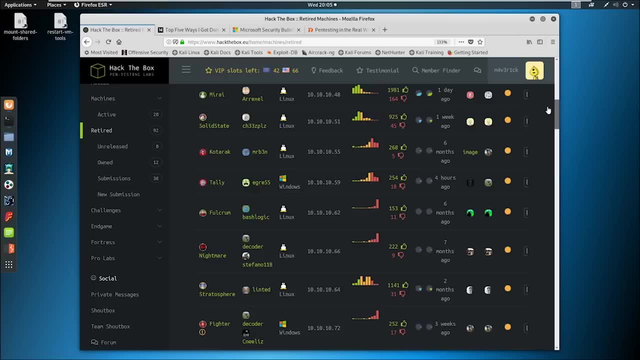 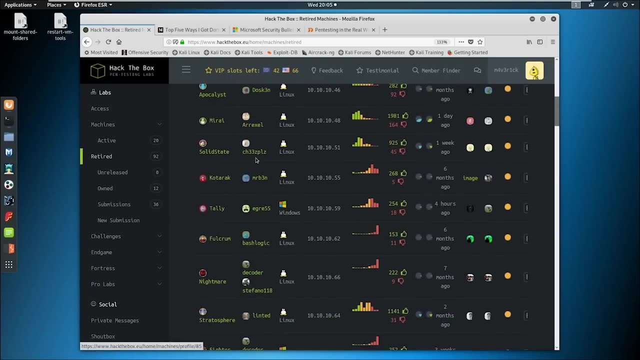 last week we'll we'll do something fun Other than that. let's go ahead and just dive right in. So I am on. hack the box Right here I'm on the tab, if you go over the left side. I clicked on retired And now you can. 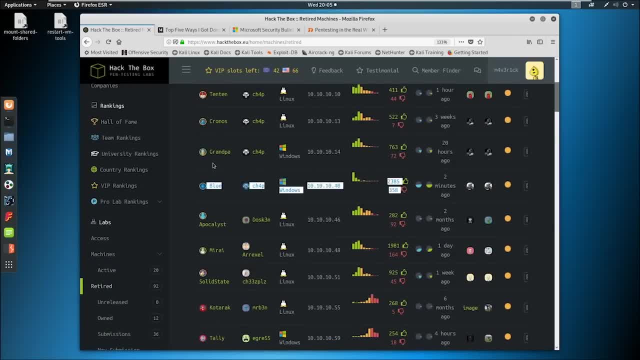 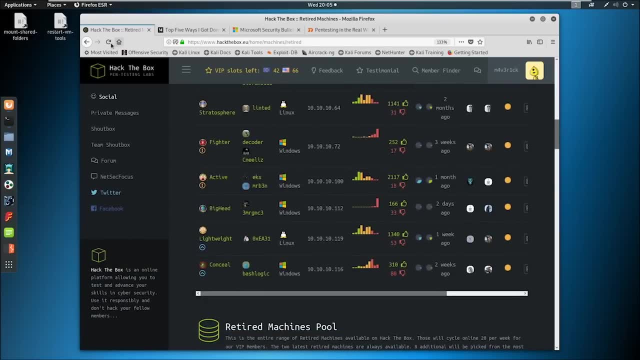 see that last week I asked you to vote for blue, which you did, thank you, And I asked you to vote for active, which you did, thank you. I've gone ahead and just recently reset both machines on my network. If you're on VIP, you're gonna be able to follow along. If you're not, you're just gonna. 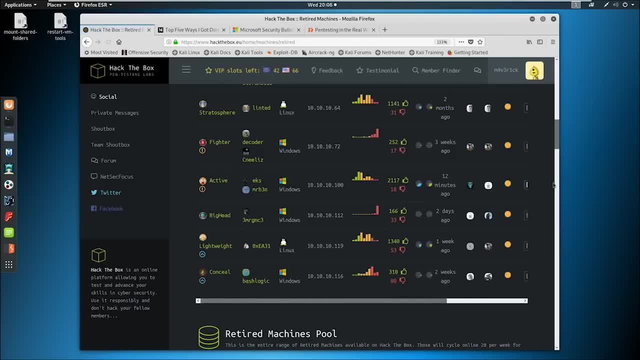 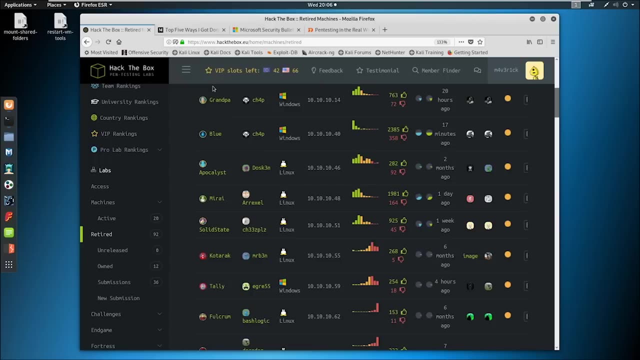 have to watch. So with VIP there are different segments of the VPN, So hopefully my resetting of the box is on a different segment of yours. But you can see I reset active 12 minutes ago and blue was reset 17 minutes ago. So for time saving purposes, what we're going to do is we're going to scan both of 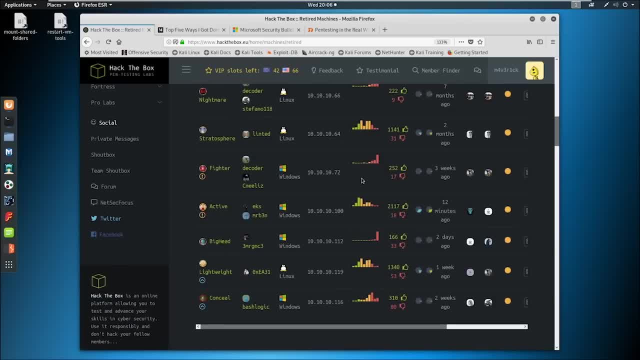 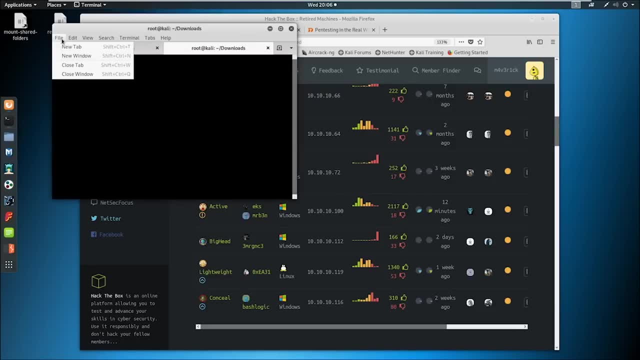 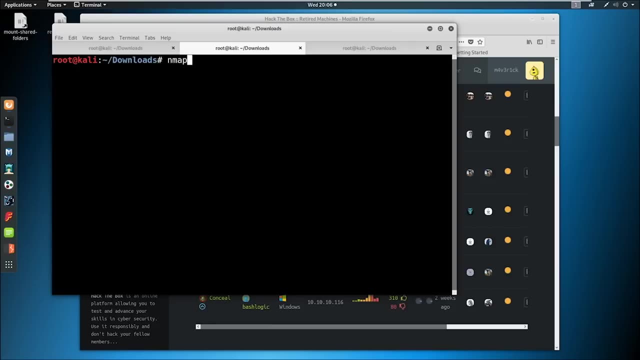 these, And then we're going to work on blue first and then work on active seconds. So let's go ahead and just get our scans kicked off- I'm not open up to New tabs here- And get these blown up, And then we are just going to end map these suckers And 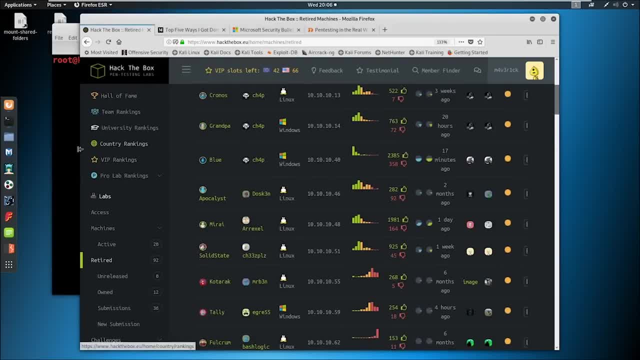 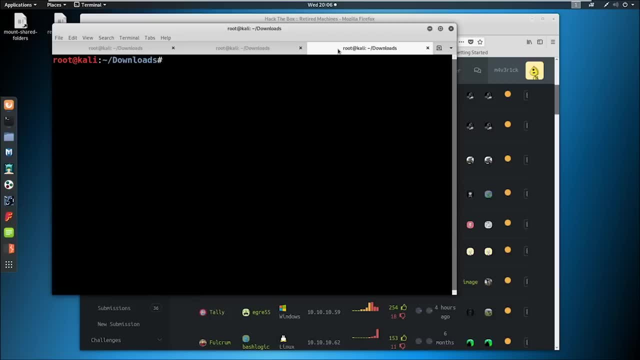 blue sits at 10.10.10.40. And active is at 100.. IP is down Nice. So I've been having issues with active today being consistently up or down And it looks like looks like blue is down as well. So we may have to give it a second, May have to toggle connection. Hopefully you're having a little bit better luck than I'm having. 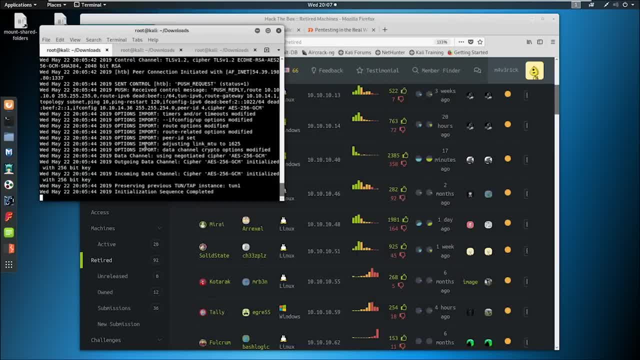 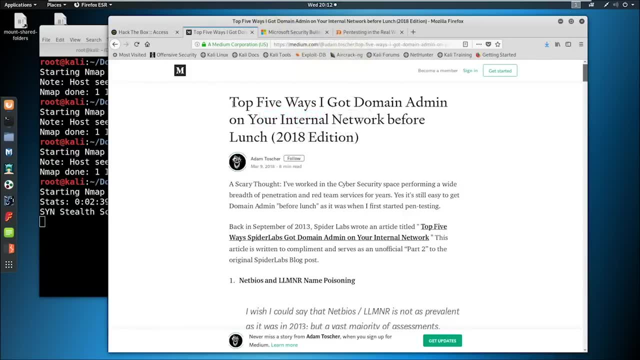 Let me toggle my connection Here, All right. So if you recall, last time we said I gave you this link, I've been giving this link throughout the course, Right, And it's been the top five ways I got domain admin on your internal network before lunch. 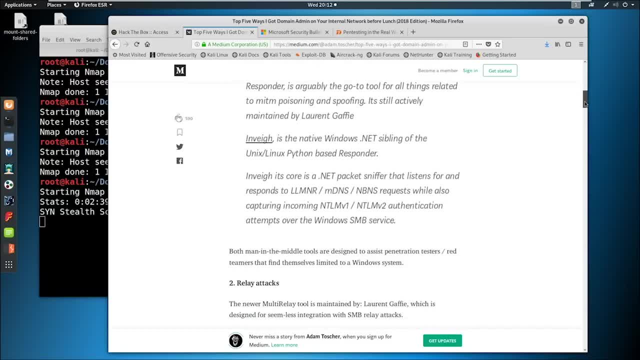 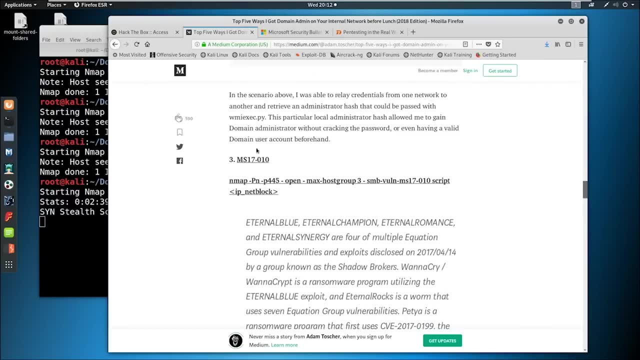 We've talked about LLM and our poisoning and net bios poisoning. We talked about relay attacks. We keep scrolling, Okay, Ms 17. 010.. That's where we're going to be talking about next. This is what blue is about. 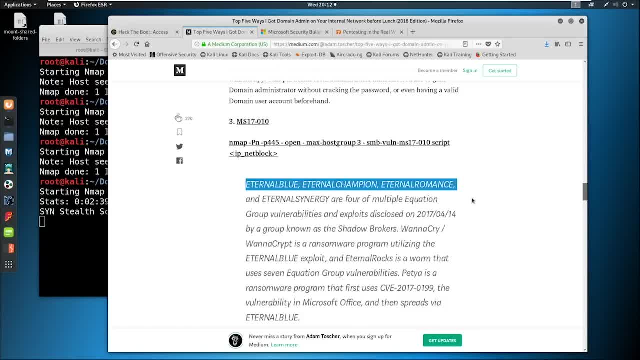 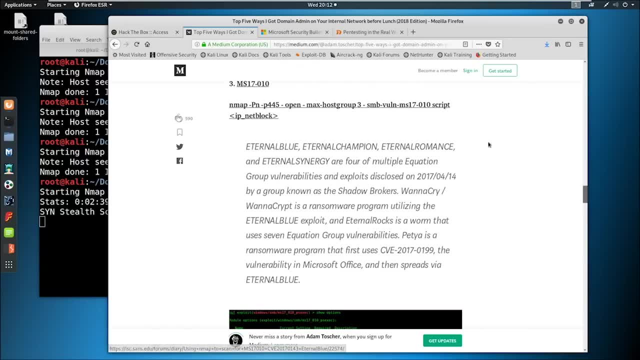 If you see it deals with the Eternal Blue, Eternal Champion, internal romance, etc. This was the shadow brokers exploit that was stolen- from the NSA, I believe- and turned into Things like the WannaCry exploit, the ransomware. Basically, It's just a A very. 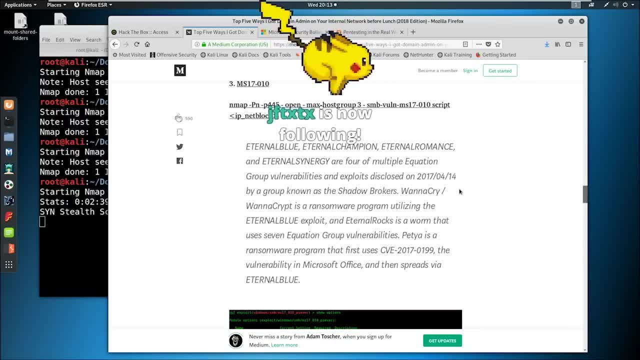 very, you know, nasty exploit that transverses your system. and this is one of those, uh, those things that sit out there unpatched on a lot of networks, mostly internal right, if you see this on the external, and it hasn't been exploited yet. very unlikely. but um, internal networks, leave this all. 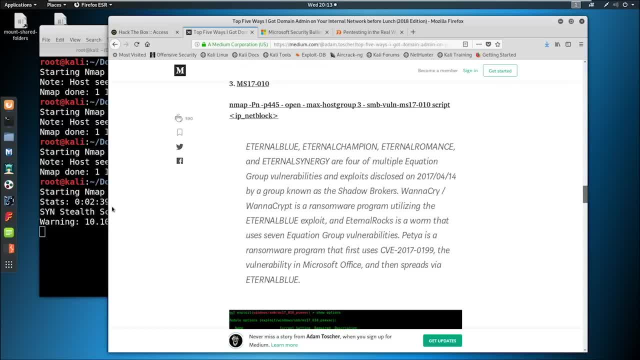 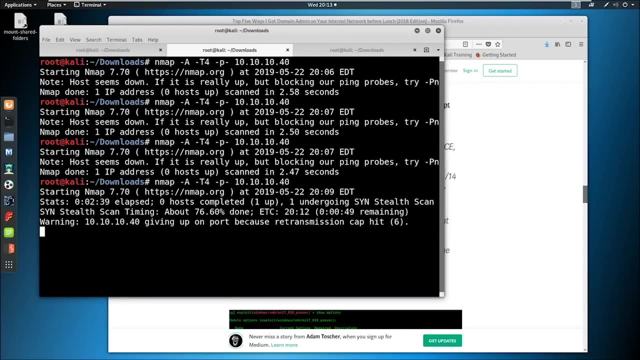 the time. think about a machine that's running some sort of legacy software that can't be updated off of. you know certain windows version people are just lazy on their patching. for whatever the reason, this is still sitting out there in a lot of networks. so let's see where we're at 99.99. 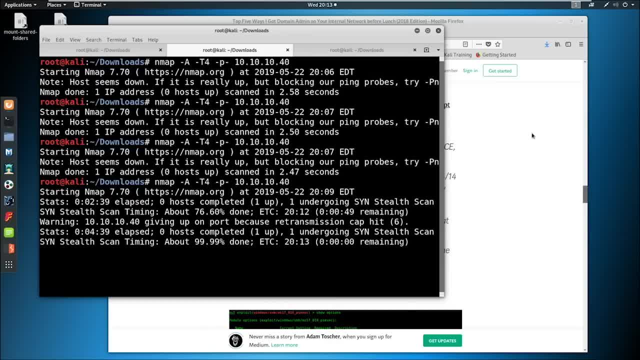 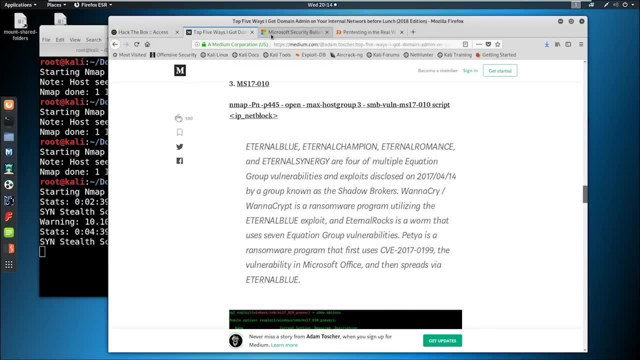 so we're going to review the scan and see, um, not only, not only what we're going to be exploiting, but we'll talk about what we would see, just from a pentester point of view, what is interesting to us with this scan. um, if you want to pull up, i've also got the security bulletin here for ms-17010, if you scroll. 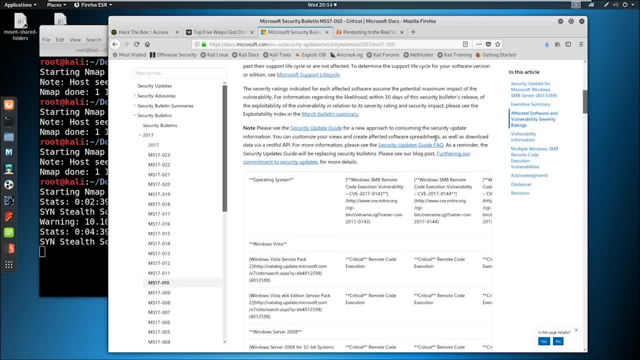 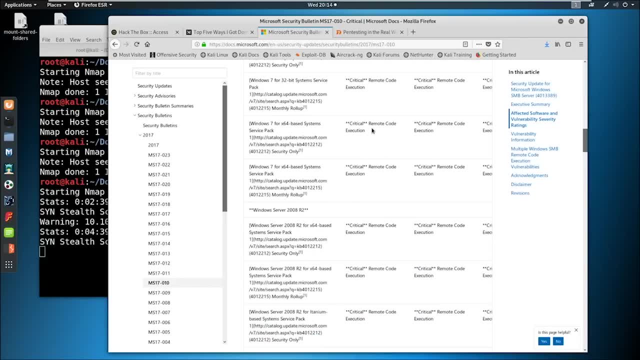 through it. you know it talks about that. it's an smb exploit. it talks about all the operating systems that are vulnerable. it's pretty much most of them. the initial exploits that that came through were for, like windows 7 and windows 2012. um, there's certain service packs that are exploitable. 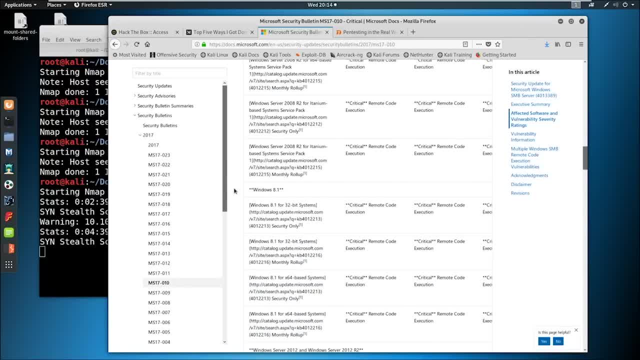 like service pack one and you, you start, you know, looking through these and you see, oh, windows 7, service pack one that is. you know, that's interesting, Maybe I should see if eternal blue or ms 17010 is on that right. And you same thing with like Windows eight or Windows 2012.. I think 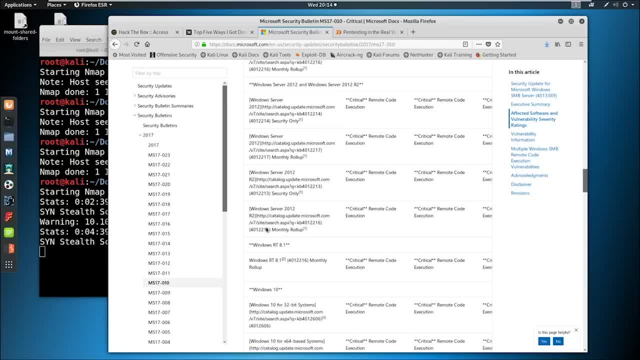 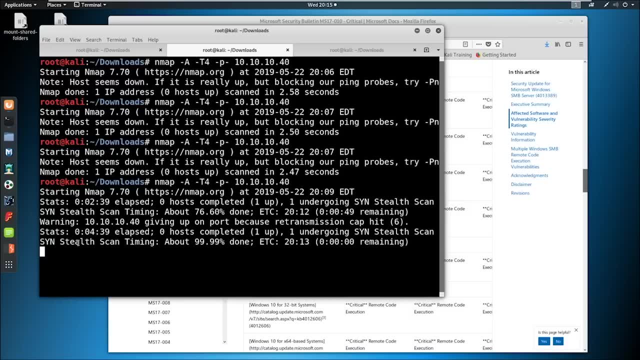 it's r2.. You, you look through these and you say, yeah, see r2 on here And you just want to know. you know what you can exploit. So I'll show you how to confirm, before we actually run an exploit, that it might be vulnerable and what steps we're going to need to take as well. 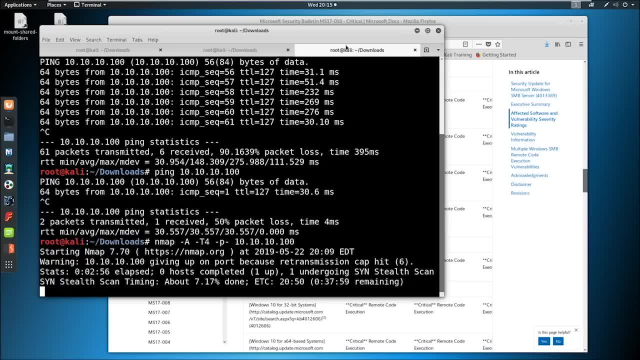 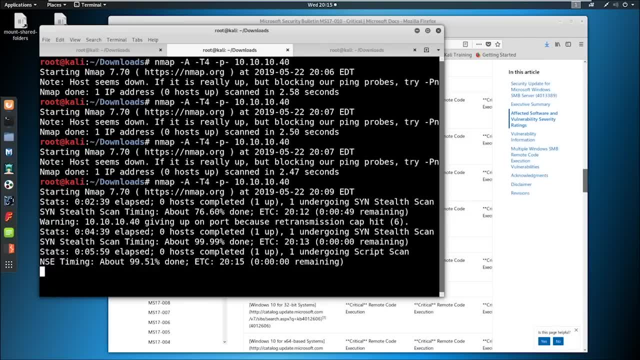 And this thing really likes to sit at 99.. Let's see, we're at over here as well. 17%. Somebody asked: how does it get infected if it's not exposed internally? So the big way that the ransomware gets in is typically through phishing. 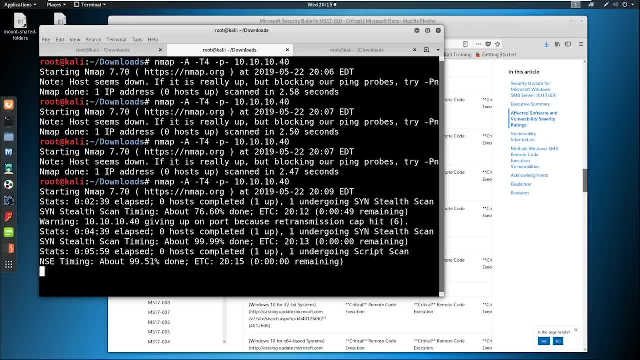 So if we're talking like WannaCry- I've experienced WannaCry firsthand as a as a help desk person. that was fun. So I mean you, you, basically anybody who opens a malicious file- that file is going to download on the computer and then it's going to start. 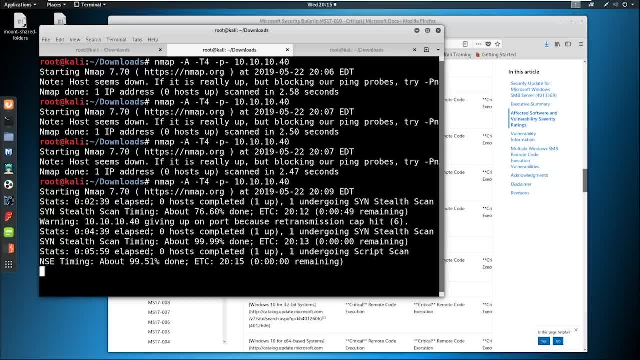 searching through the network. right, It's going to look for SMB open. if SMB is open, it's going to try to navigate to other computers through the network and exploit as many as it can. it'll start encrypting the files And you know that's how you, you know you- can get the files. 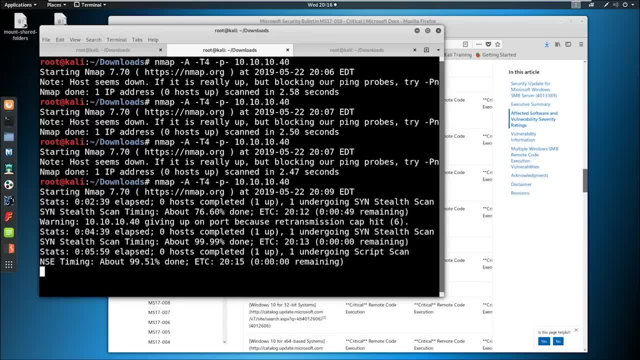 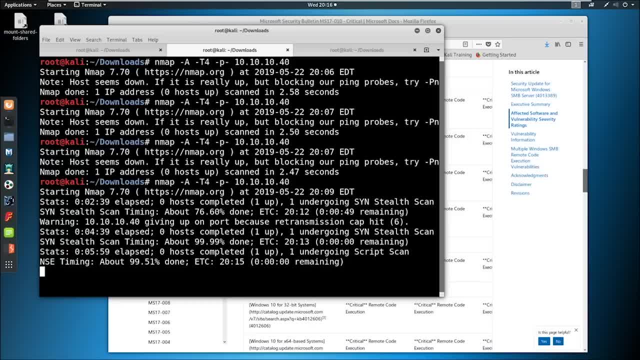 you're on the network, regardless of how we got on. So we've been assuming internal network access for three weeks now. So, regardless of how you're in the network, these are one of the easiest machines to drop. We'll see what it came back with. 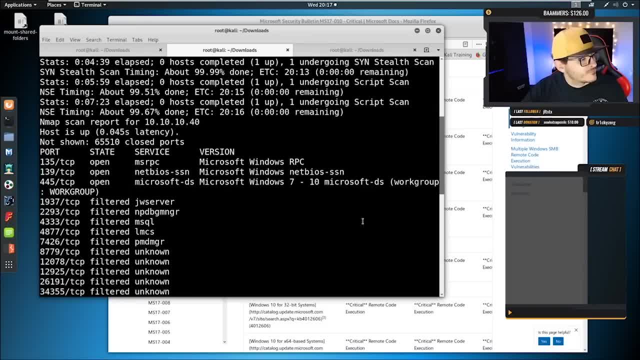 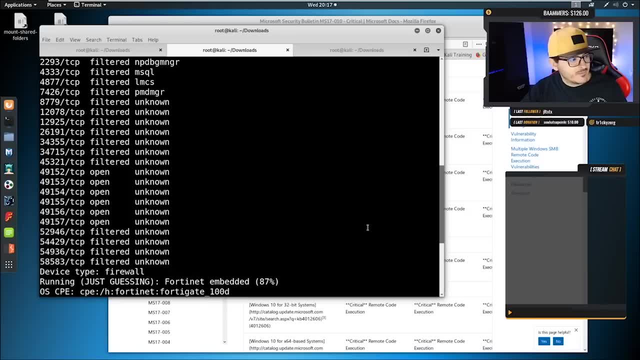 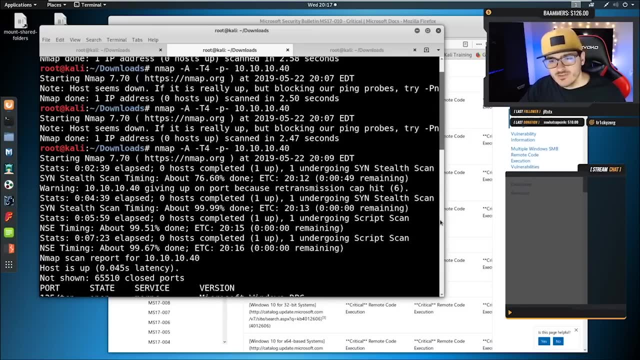 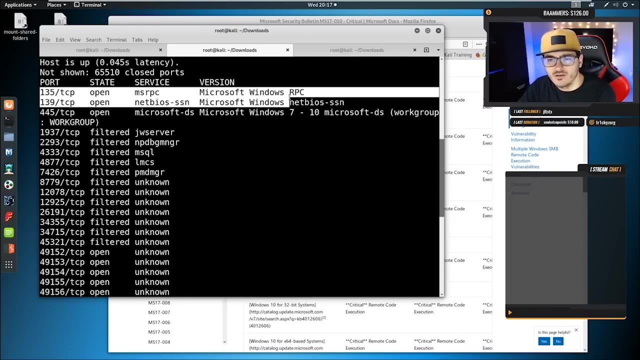 This really didn't do a good job. Your scan is likely going to look way different than my skin is. Typically when I've scanned this before and run this before. it gives us quite a bit of information on on what's behind, not only port 139, and port 45. But it'll still. 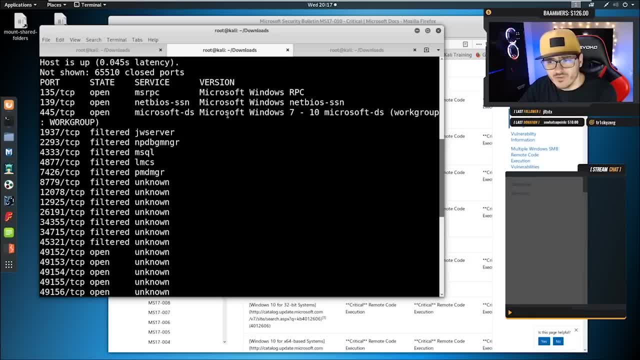 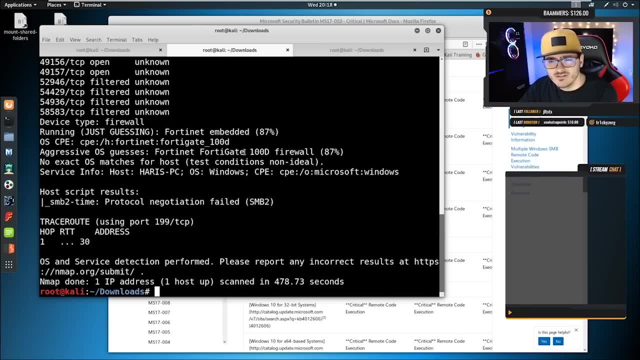 say what service type we're running, It'll say: you know. it even tells us, I think, the name: Yeah, like Harris PC, you would see more than that. For some reason it's picking up that like there's a Fortinet firewall. I don't know what's going on with a hack the box tonight, But this is. 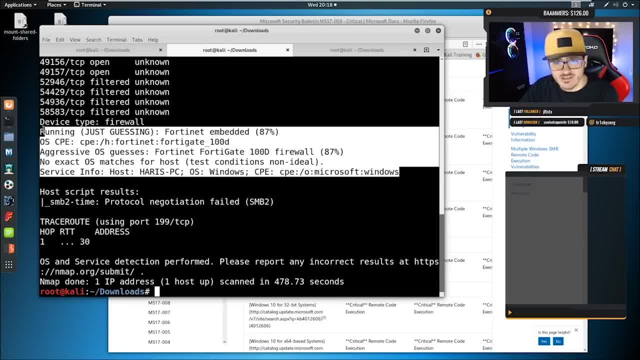 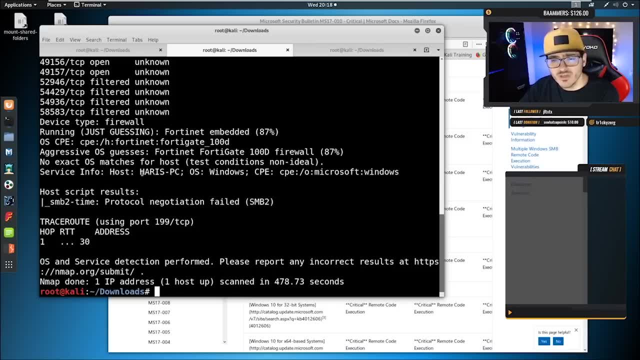 all this is probably not going to happen to you, I'm just getting unlucky. So typically we have some script results down here that will tell us a little bit more, also the information that it picks up. It should be pretty much the same. 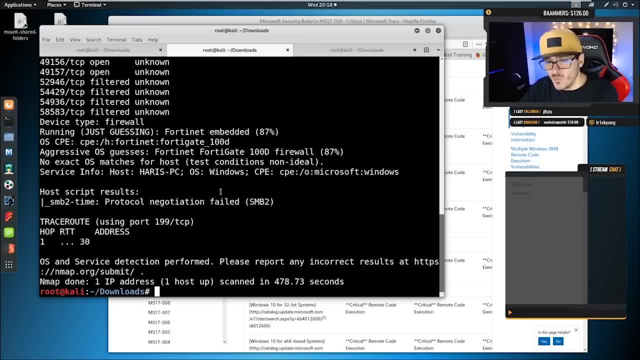 should be picking up some sort of Windows information in terms of OS. the SMB is going to tell that out. So really, that's we're going to look at. there's another thing on here, to where SMB was unsigned. If you see that that's obviously a finding, because we can do relay attacks like we. 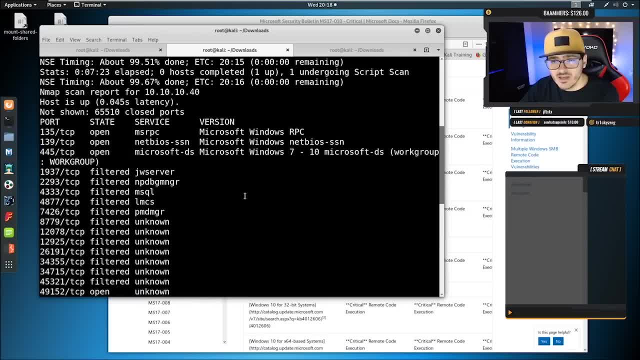 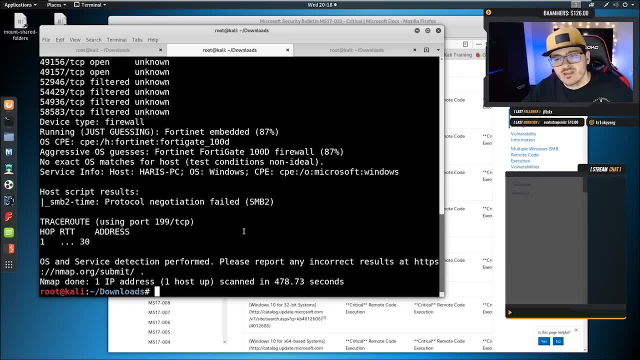 talked about last week. Unfortunately, it's not. It's not working out for us. So what we're going to do is we're going to pretend that we saw the scan, and the scan came back with some information And we have deduced that 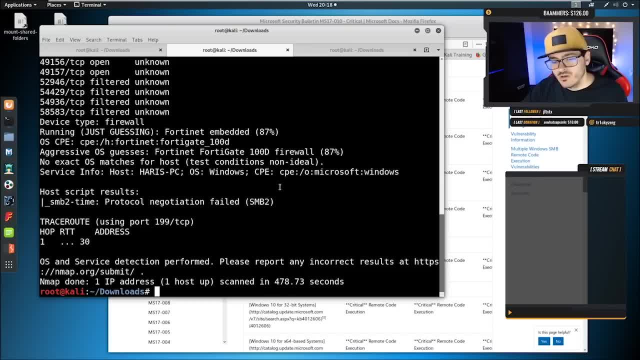 And we have deduced that the scan came back with some information, And we have deduced that the scan came back with some information And we have deduced that there may be a potential exploit here. So one of the things you should do- and if you're running Nessus, Nessus is going to do this- 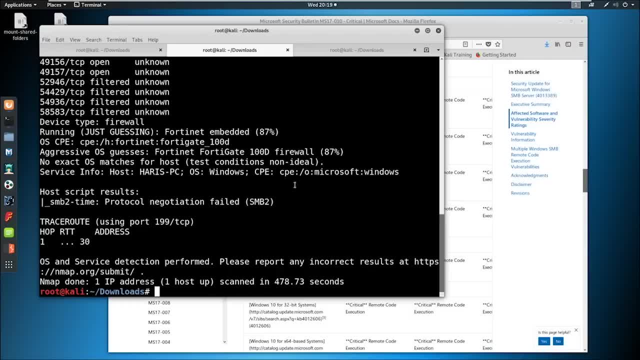 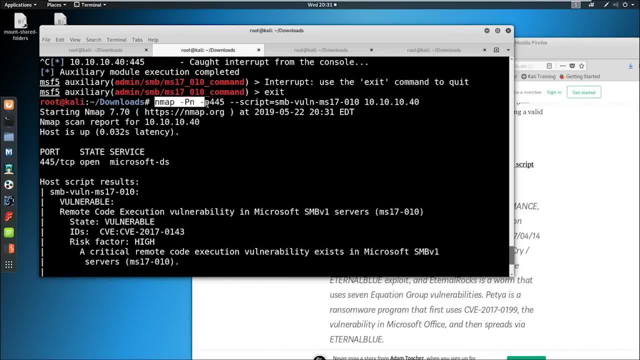 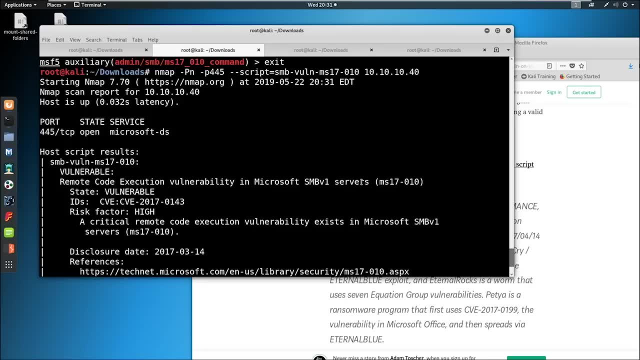 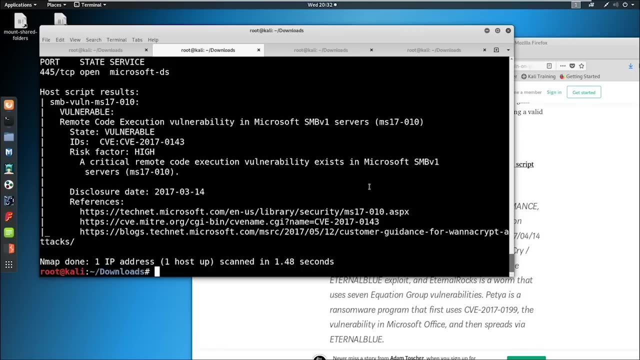 Okay, so here is the script we ran And map dash pn 4445.. Here's script And then it spits out: Hey, looks like it's vulnerable to this remote code execution. right, And if we were to rescan we'd. 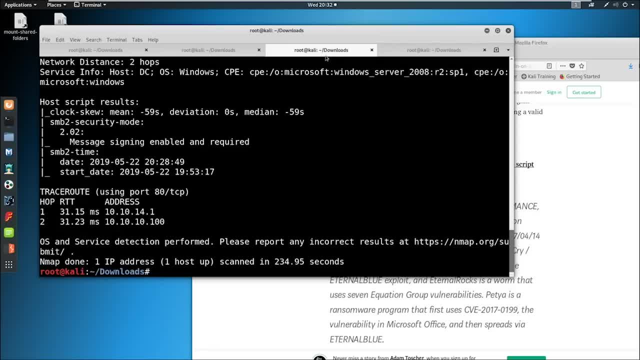 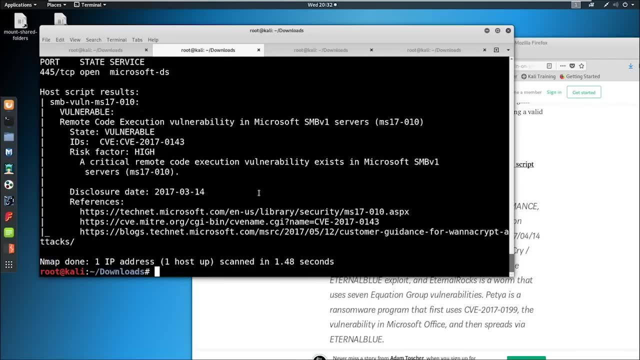 probably see more of the map this time around, And we did. we get it back. our- Hey, we actually got back our scan for active as well, Cool. So we've got this scan here saying it's vulnerable. So at this point, if we're a pen tester, we've got a couple options, depending on what the 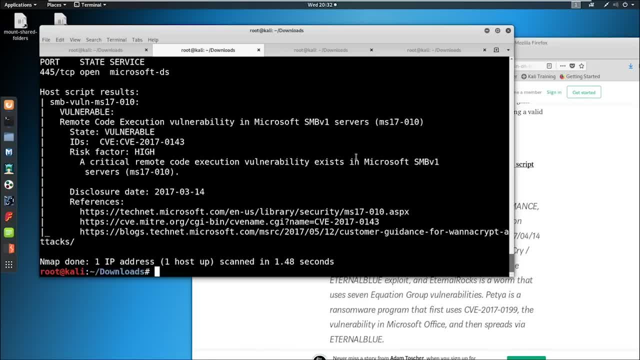 client has told us right. If the client says, hey, you have free reign, go ahead, do whatever you want. Or if the client says, hey, you know what, before you run any crazy exploits, please let me know, because an exploit like this may actually take down a system, it may mess. 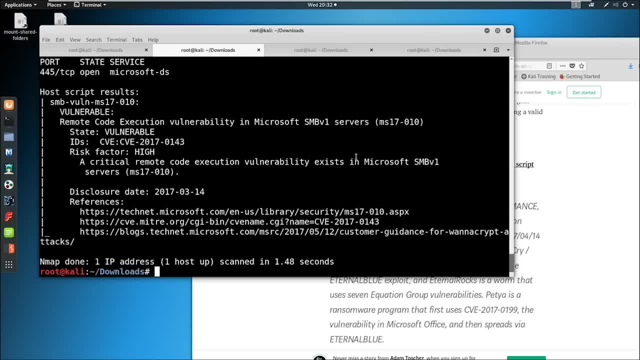 things up depending on what the system's doing. if the system's some sort of critical infrastructure where it can't go down, you might not want to run that exploit right. So it's important to know on these RCE exploits that you're probably better off being safe. 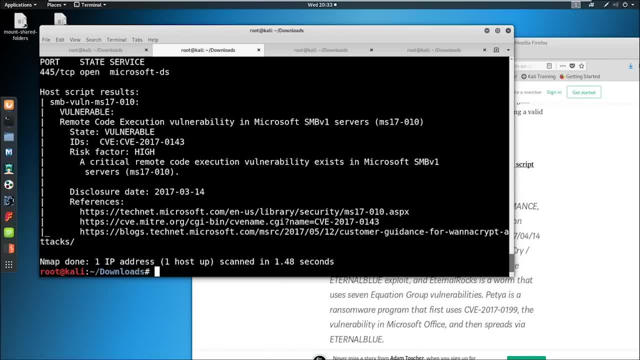 than sorry, and you don't want to take something down that's critical and have a client pissed off at you. So you call the client. You call the client up, The client says, okay, fire away. And that's kind of where we're at here with this exploit. 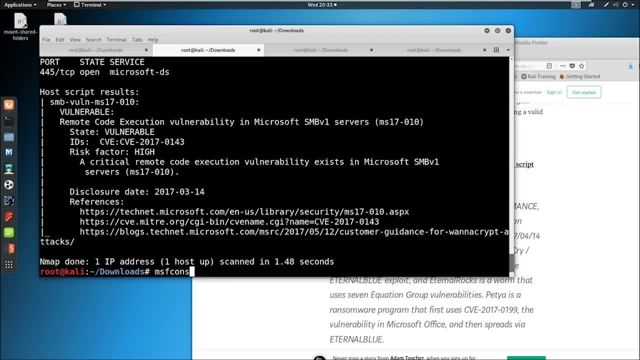 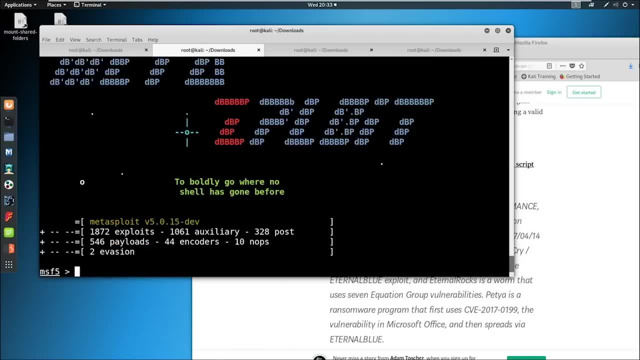 So if we come in and we say, let's go back into Metasploit, And I don't think I'm thinking, guys, this stream is not going to make it to the live cut. So what we're going to do, I'm probably just going to piece together a couple of my old 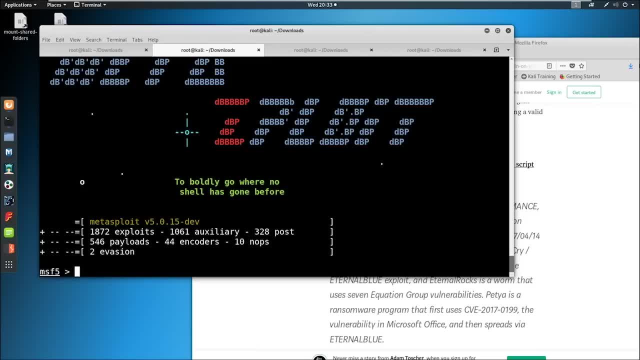 streams that I have on these topics and throw them in as a. as a. you should have been there for the live shit show And we'll. we'll just call it off. We'll just call this a special night. So we've got MSF five. 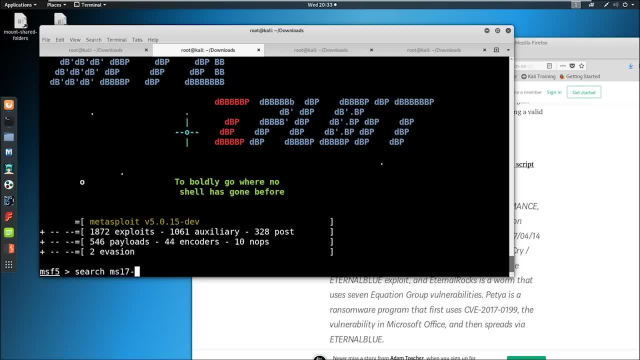 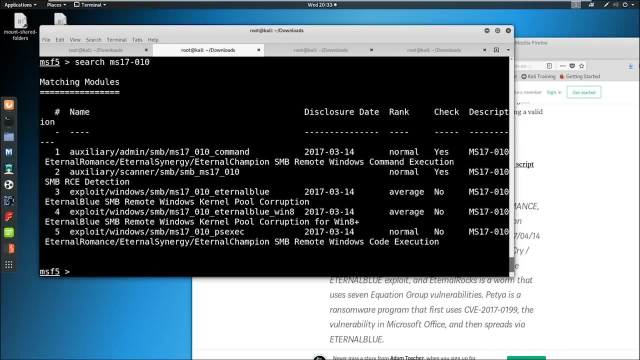 All right, Let's say search MS 17 0 1 0.. And we are looking for a exploit: windows SMB MS 17 0 1 0, eternal blue, right here. So you can just copy this bad boy and paste it. 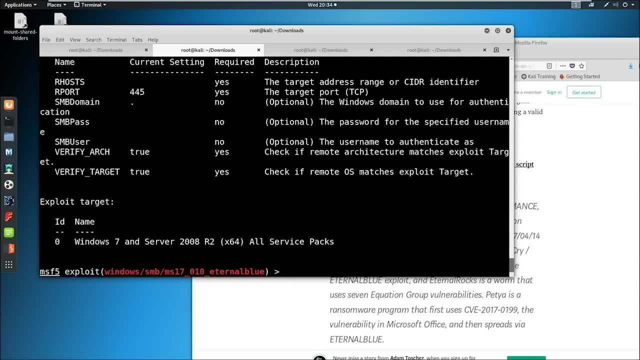 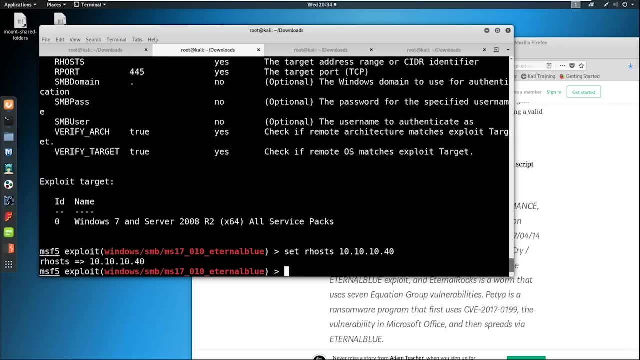 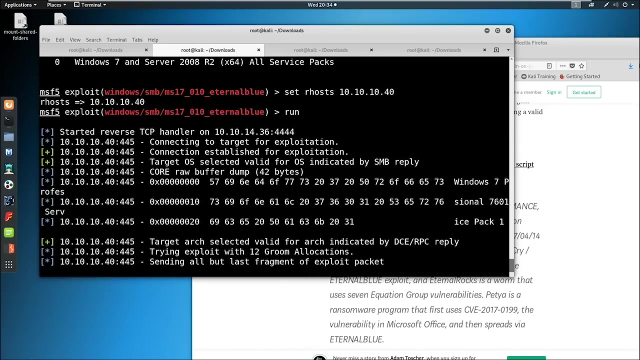 We're going to set the our host to 10 dot, 10 dot, 10 dot 40. And then we are going to run this. now a couple of things to note. First thing note is this might not work on the first try or the second try. 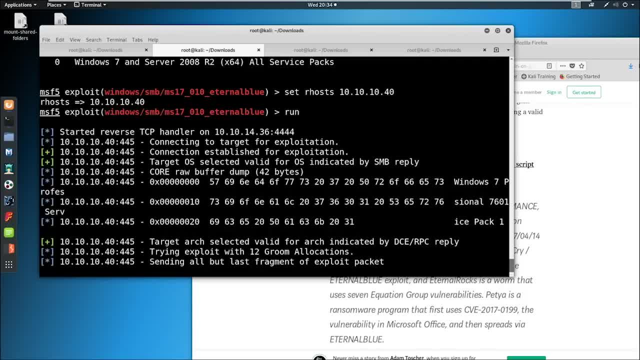 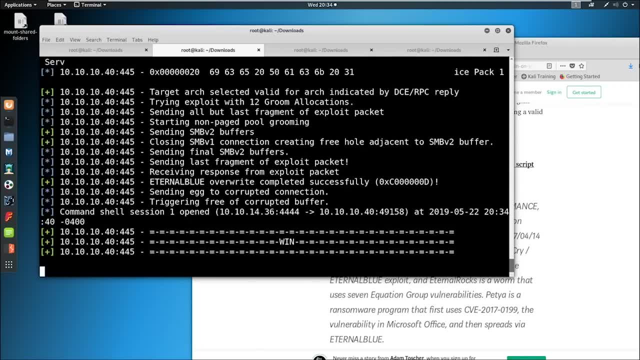 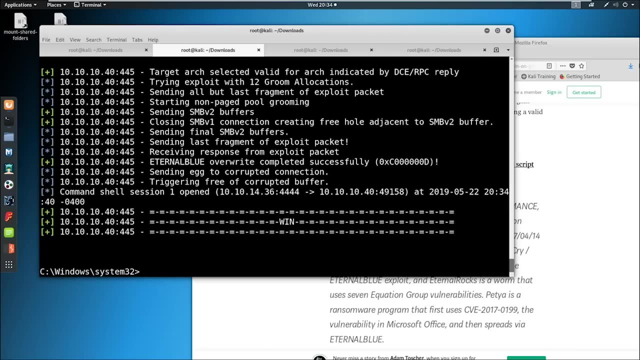 It might take a few tries to actually work. Okay, Uh, you know this is very, very tricky exploit to get running. Of course it runs on the first time, gets us win. Next thing to note, it puts us right into a command shell. 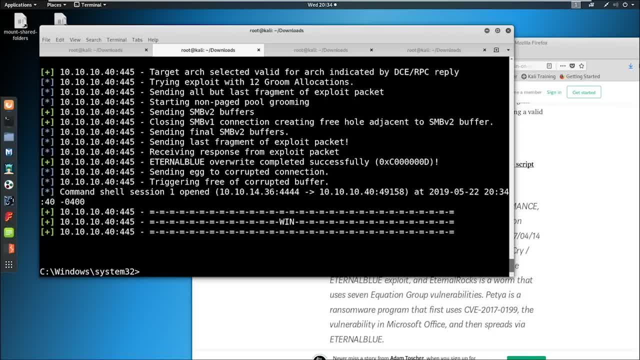 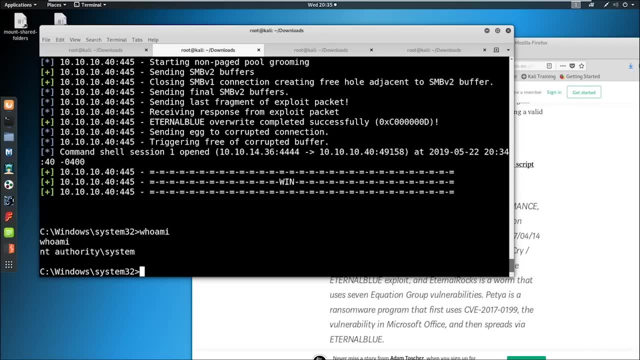 So if you are a meterpreter fan boy, like I am, this is not the best situation we can approve upon this right. Um, so this is just a generic payload. Uh, we can say who am I, And it puts us in as authority system, which is great. 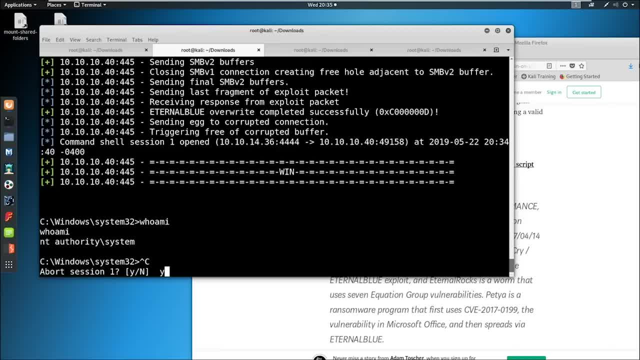 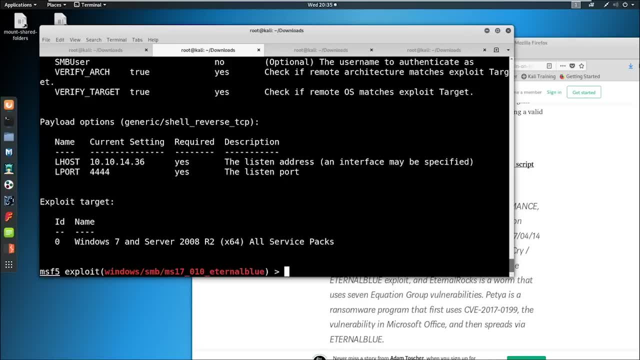 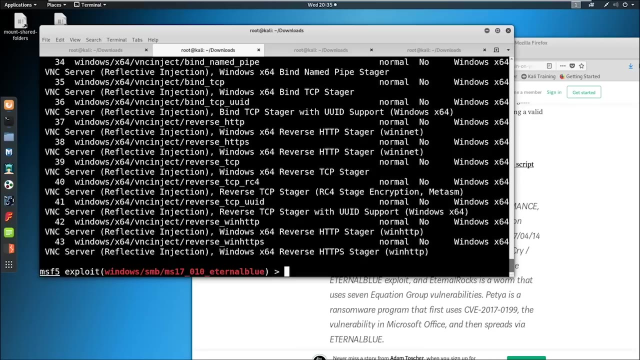 Um, but let's control C out of this and just say yes. And let's say options again. this time we can see the payload option says generic shell, reverse TCP. And we're just going to say how about we say show payloads and see what's available? 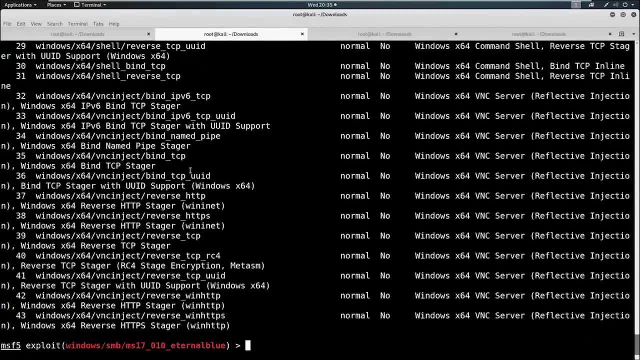 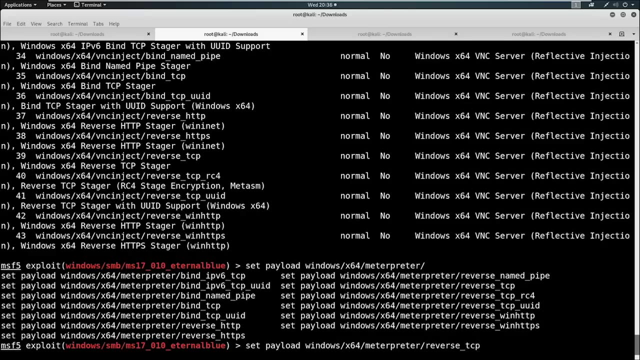 to us. We've got 43 payloads, but I'm going to use a windows 64 bit meterpreter. So let's just say: set payload, windows 64 meterpreter and then let's just double tab to see our options. Uh, reverse TCP is probably the best bet here. 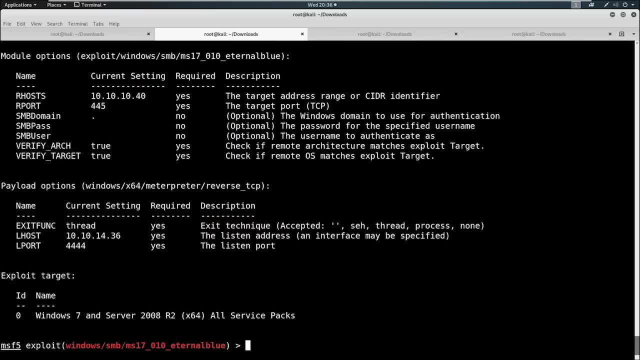 Always good to double check our options as well Once we set the payload. We want to make sure That our L host is still holding true. Our L port is also still holding true. Sometimes it resets these down to nothing, or if you've got an exploit running which. 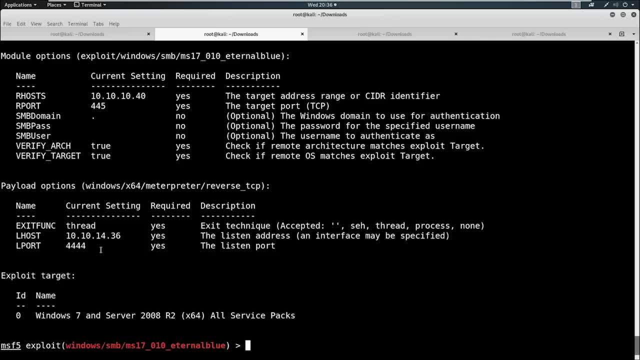 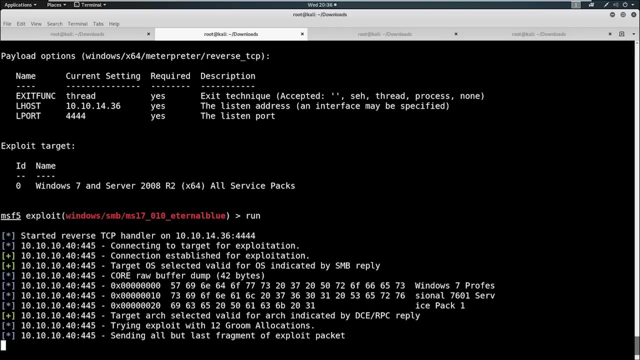 is sometimes the case already on a port. it might default to this four, four, four, four and you might want to set it to something else. All right, So now let's go ahead and run this again. Let's see if we get lucky twice in a row on the first fire. 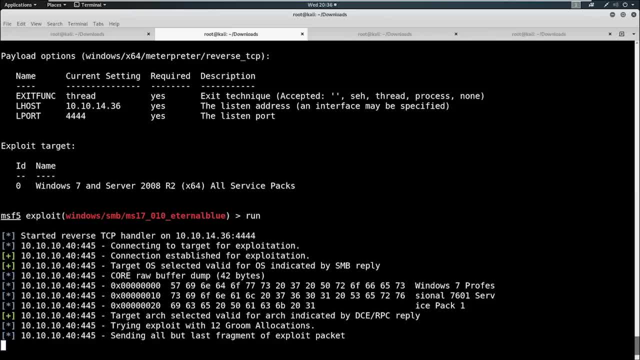 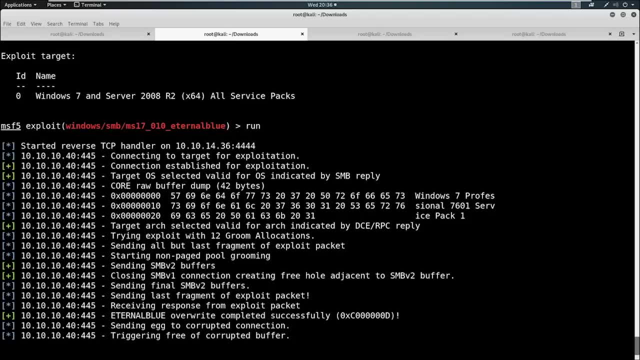 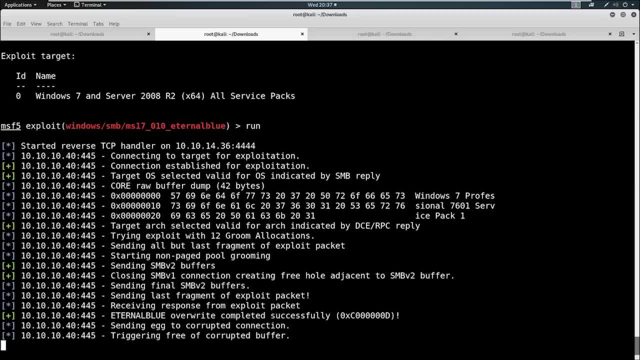 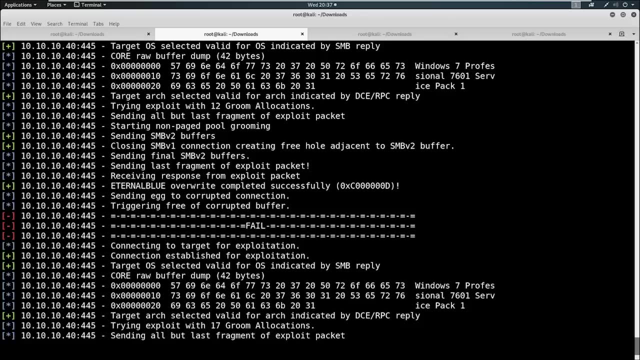 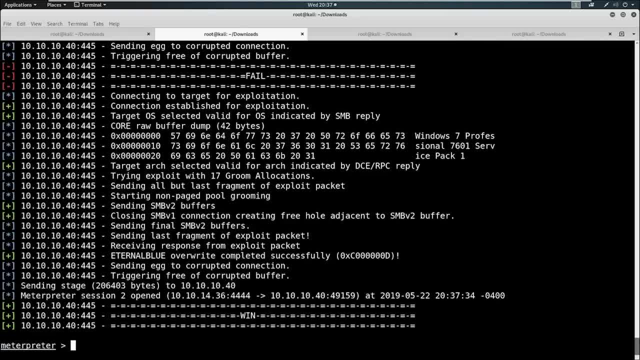 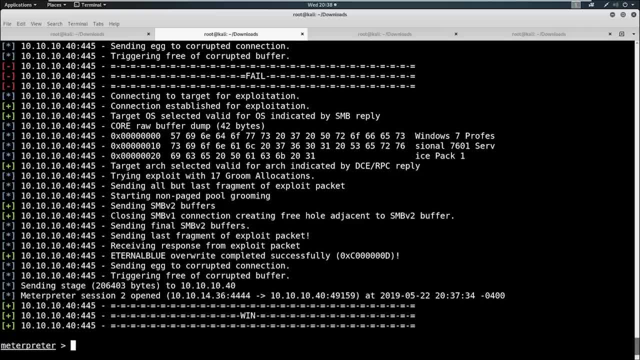 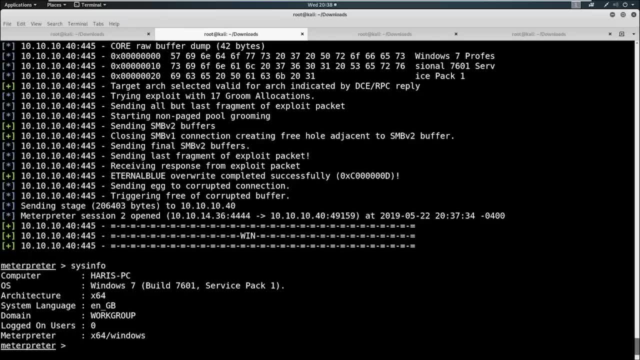 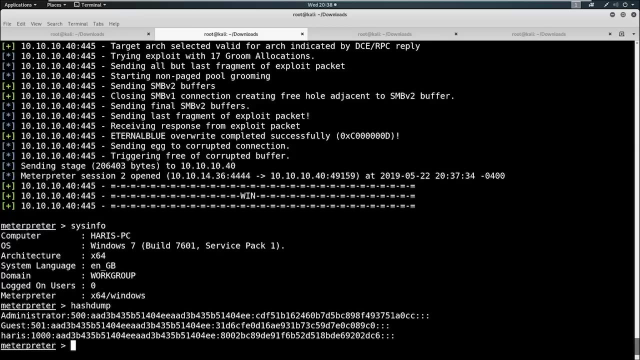 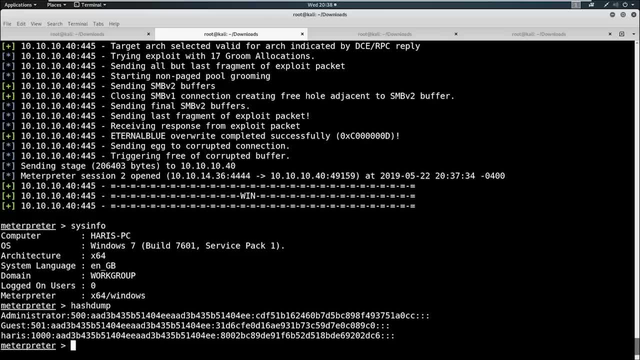 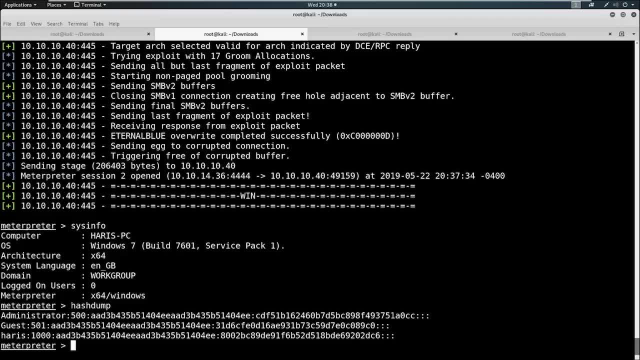 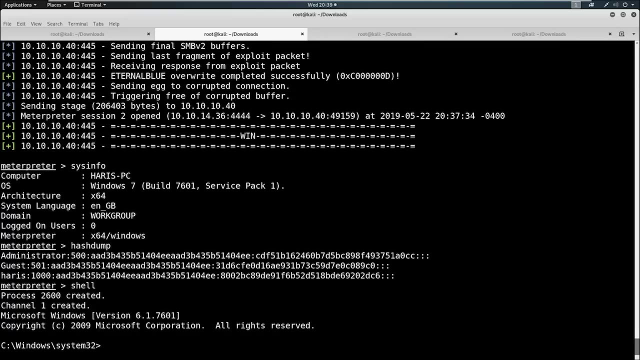 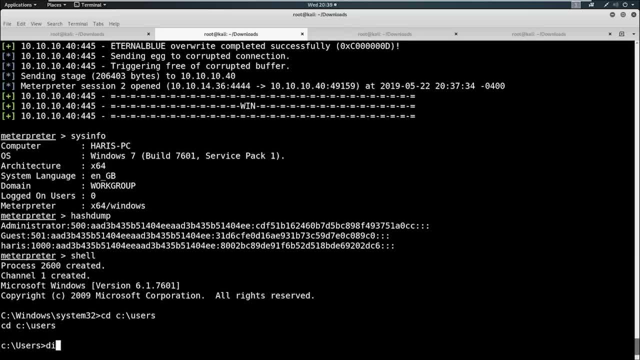 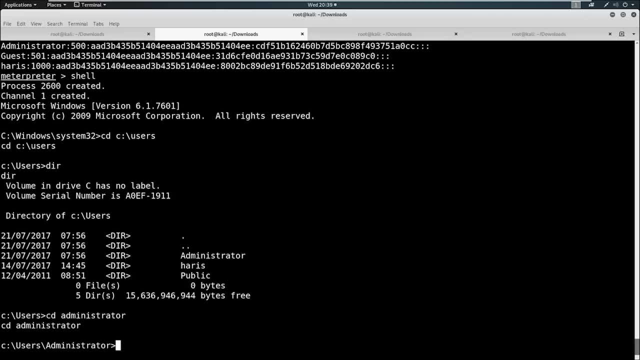 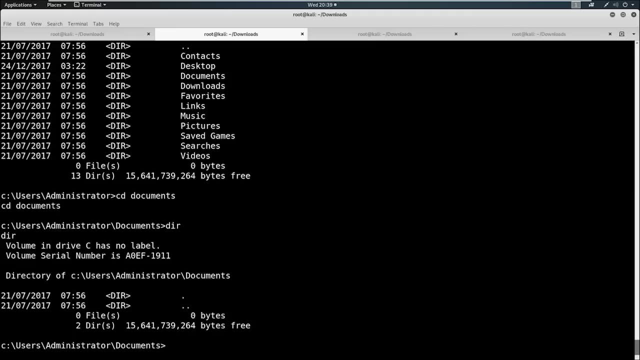 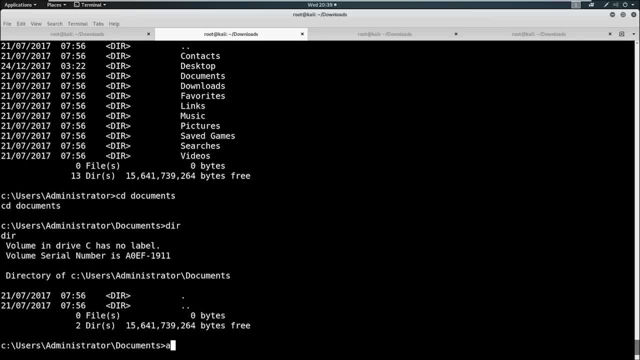 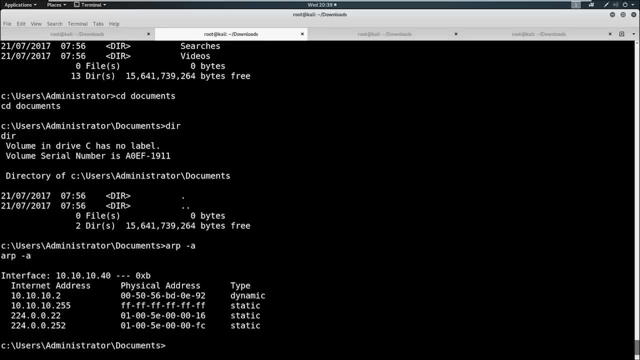 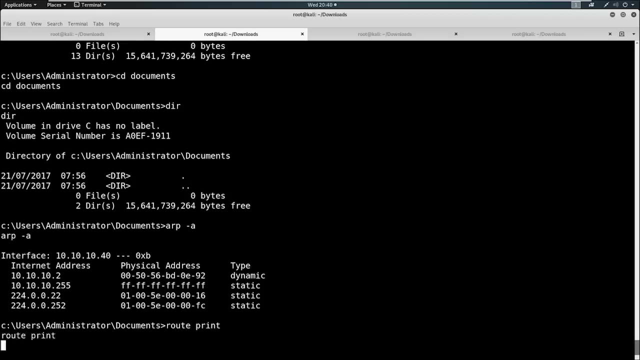 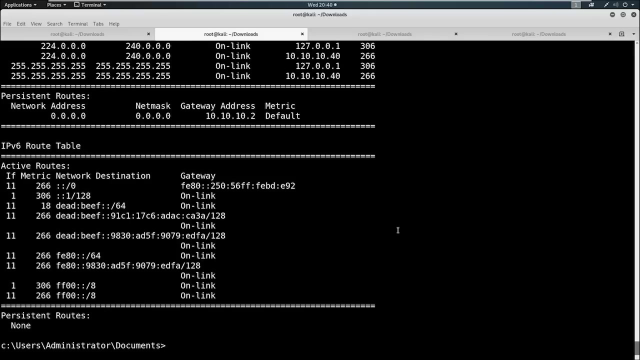 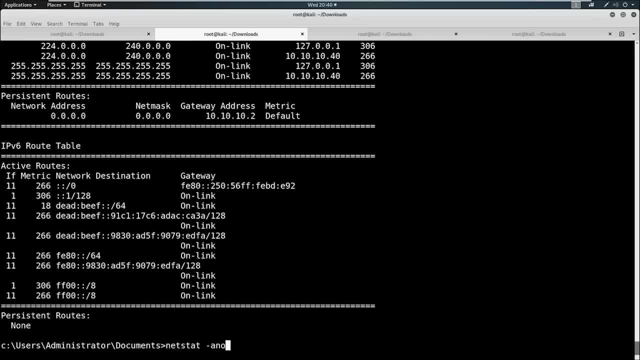 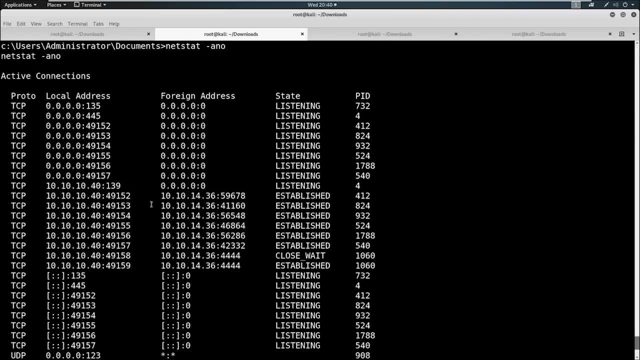 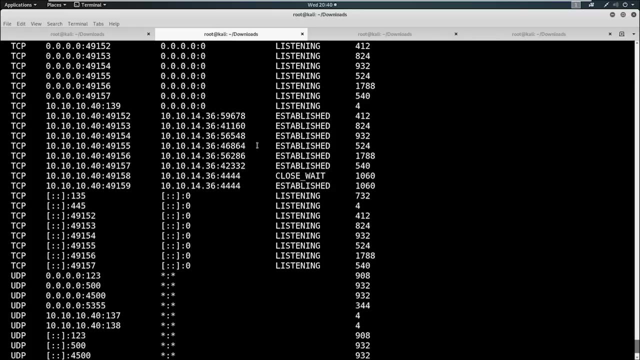 So if we go net stat dash A and O, we can look at all the connections that are coming in and going out, right. So we talked about it a little bit last week, about dual homed machines. For example, if this PC for some reason had two NICs and one NIC was sitting on a 10.10.10. 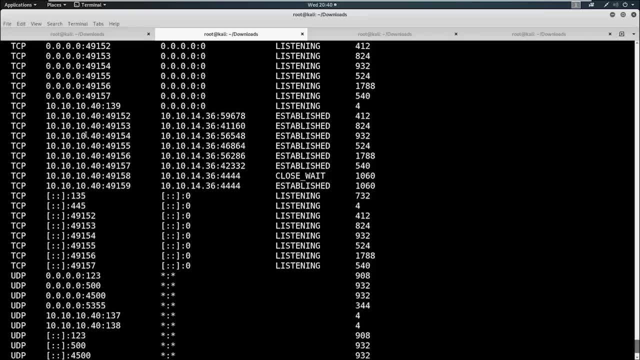 network and the other one was sitting on 10.10.11,, for example. we might be able to see that the 10.10.11 is talking to a whole different network that we had no access to, And we're going to talk about that in more depth next week when we talk about pivoting. 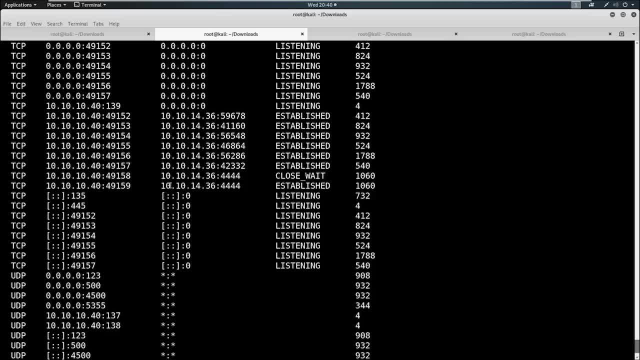 So that's a pivoting situation where we want to go into a- you know, a different network network, How we investigate these higher ports. So these higher ports, if you look at what we're doing, like the 4444 here, those are 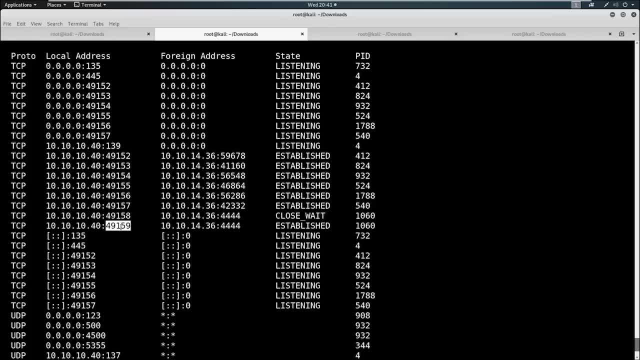 established from us connecting, So we opened a port on their end. These other ones, who's to say what they are, we'd have to see, you see, a lot of high ports like this going out of, like 443 and other, you know, like internet addresses. 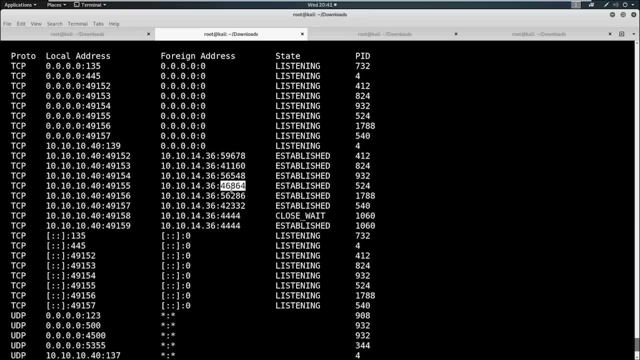 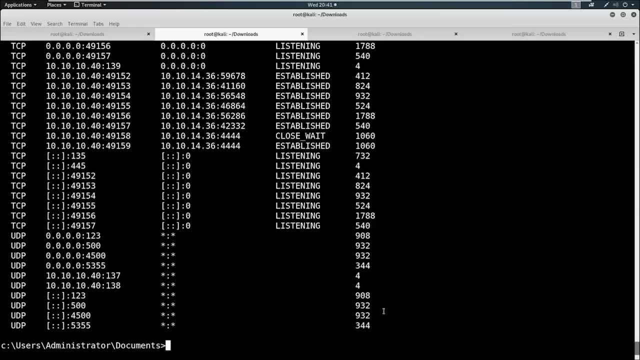 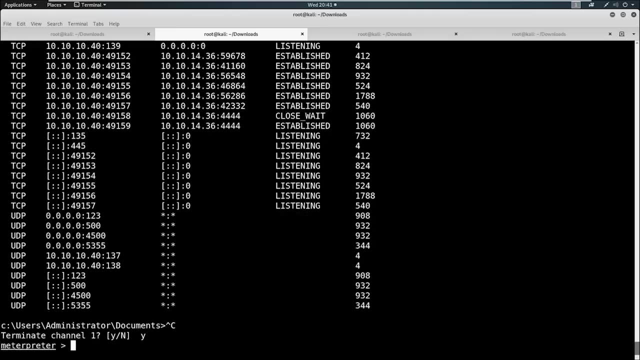 These could be other people's shells. for all We know they may have just put in like other. you know, it's hard to say without being able to go into the machine, So we want to look at those things, Of course. control C. 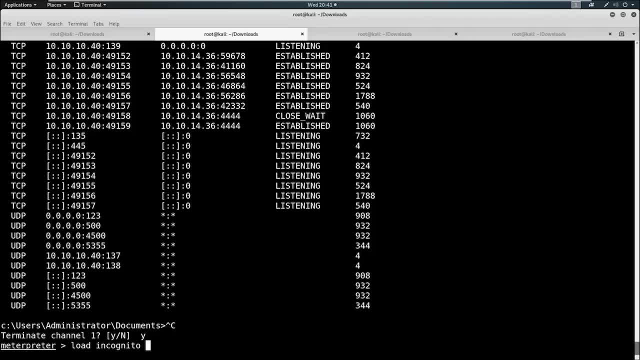 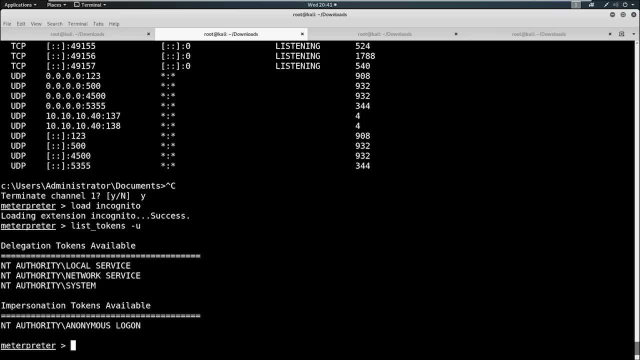 We can load some extra modules as well. We can load incognito, which is my favorite, And we just say list tokens, dash you for user? Okay. And if we're on a domain network, we may catch a domain administrator who had logged into. 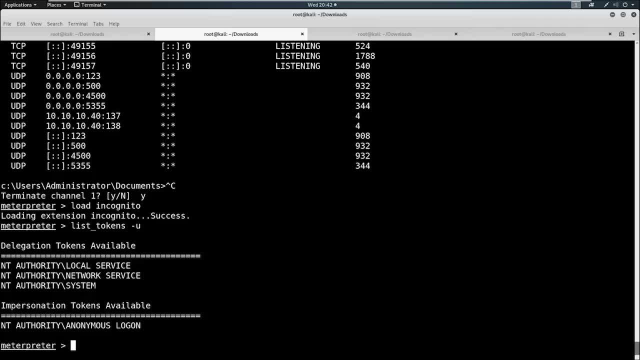 this account. Remember we talked about the tokens and how they worked last week. Obviously, there's no domain account here to log into because we're not doing that, But something to look for. if we're using 64 bit architecture, we can load Kiwi. 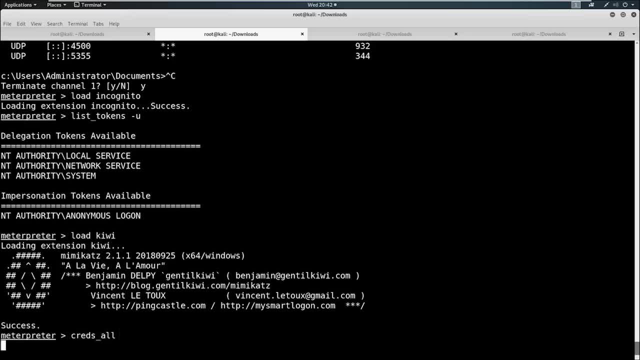 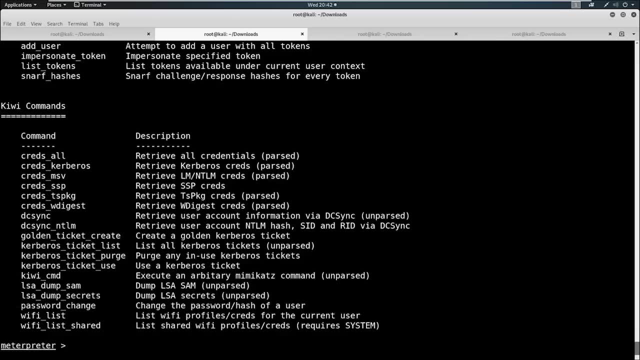 Kiwi is awesome. One of the best commands is creds all again. we talked about this last week: no creds here, But if we type in help, There's more than just the creds all we can talk: creds Kerberos, golden ticket attacks. 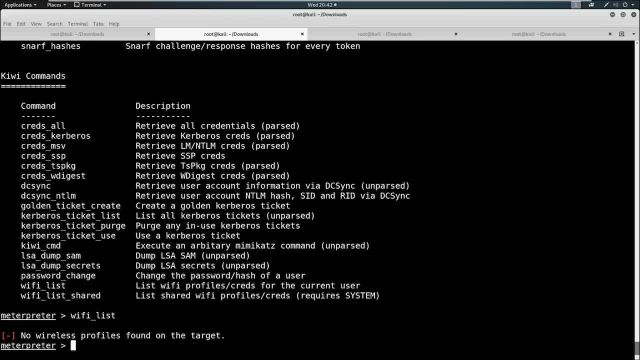 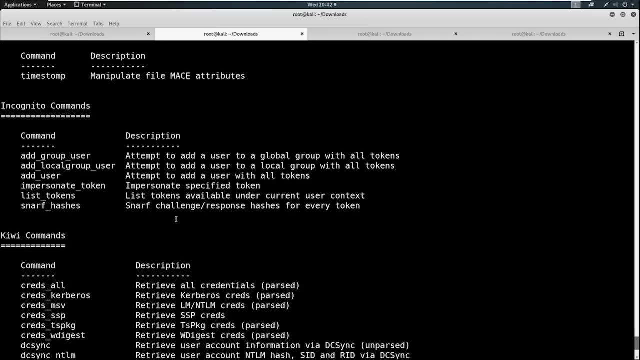 come through this. we can do Wi Fi list, that there was a Wi Fi profiles, So there's a lot of things that we can we can get just off of Kiwi. So these are some things to look for, things we've talked about. it should all be coming. 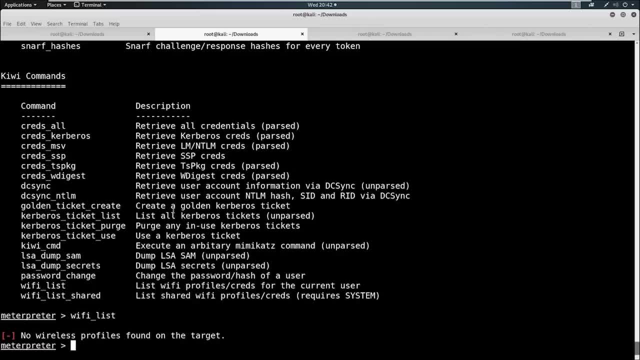 together. right, This is just a very, very simple exploit, But the post exploitation is really the most important. like we, we we own this machine in two seconds and there's a reason: it's on the top five lists. like i said, it's on most major networks. um, since we owned it so fast, we need to be able to make sure we. 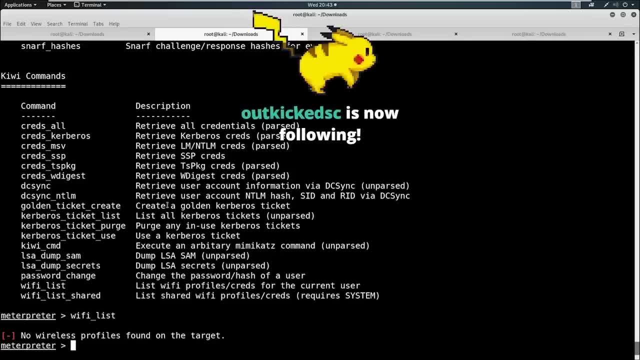 enumerate around everywhere, right, um, we're looking for sensitive files, those hashes. where can those hashes lead us? can we impersonate a domain admin? what kind of net commands can we get access to, etc. so um, every little computer has a piece to play in the final picture. it's just seeing how. 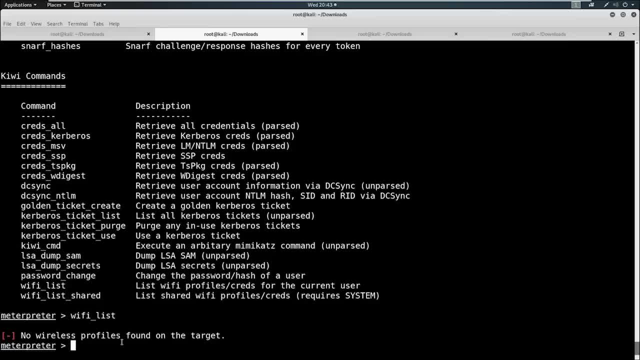 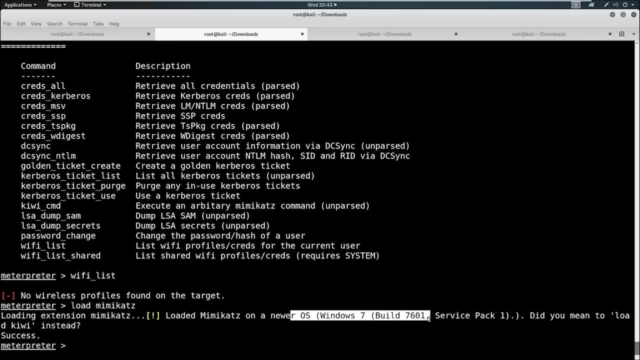 that piece fits into the puzzle. what's the difference between mimi cats and kiwi? kiwi is a 32-bit, right? so if we say load or sorry, mimi cats is 32-bit. if you say load mimi cats, it's going to say hey, you're loading on to newer architecture, right os. so we want to actually use. 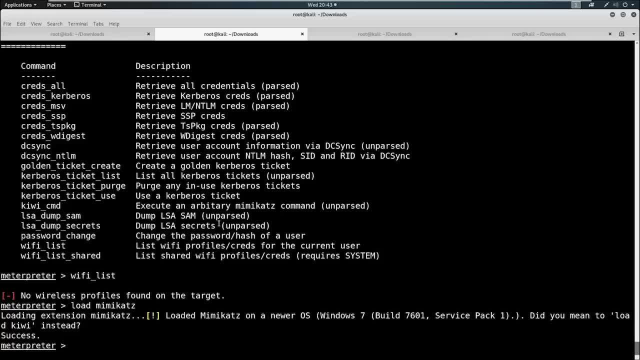 it on um some older architecture: kiwi is the newer and better mimi cats so. so all right, so we're gonna call this one a day. this one was just gonna be a 20-minute box. that's turned into 45 minutes again. i'm very sorry, guys. uh, even i struggle, you know. so, um, let's go ahead. 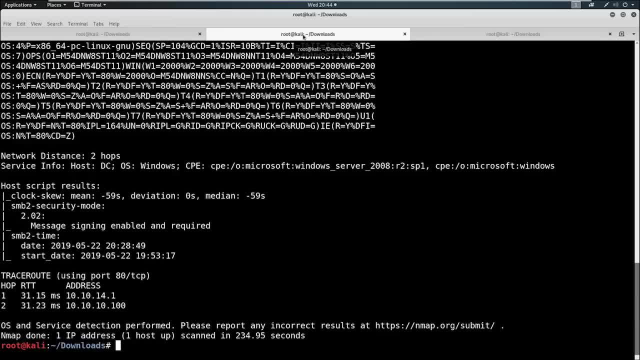 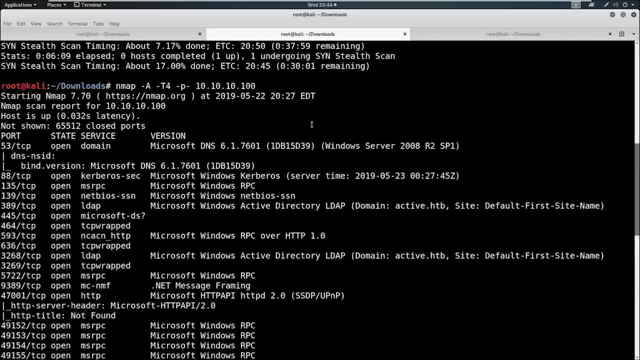 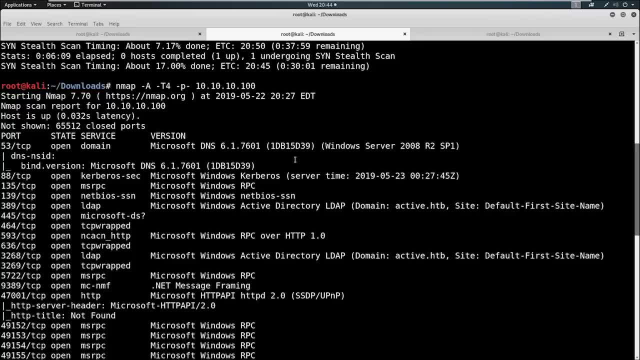 realistic. so, if we look at it, there are some signs that what we're up against is likely a domain controller. you can see that it's running dns. it's got kerberos, which is an authentication system. we've got 139 open. we've got ldap open for active directory- right that should. 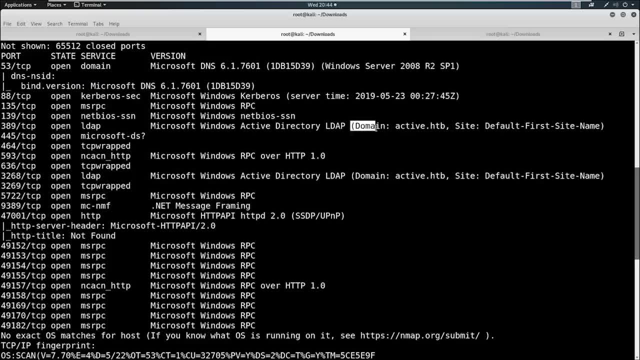 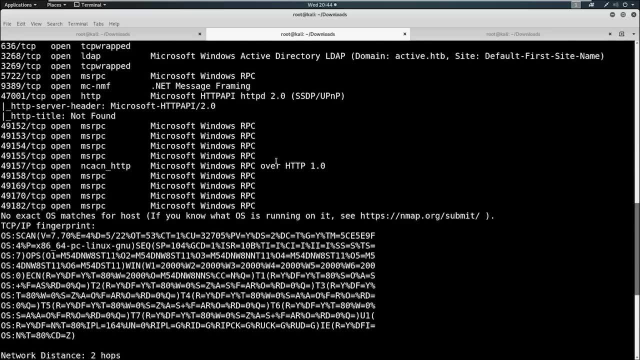 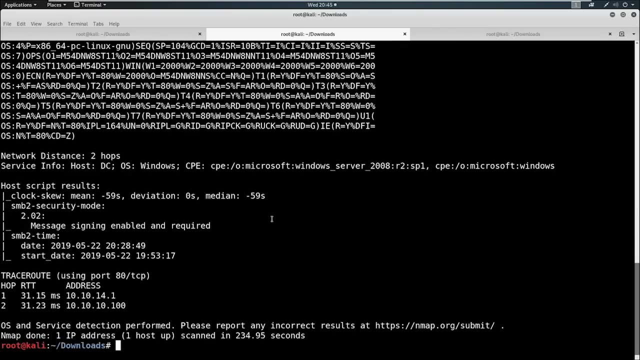 be a pretty big sign that we're running a domain, and the domain here is active, dot, hdb. we can go through all the ports here. it's very, very similar to that, like i said, of a domain controller. so when we see this, we look down here: smb and 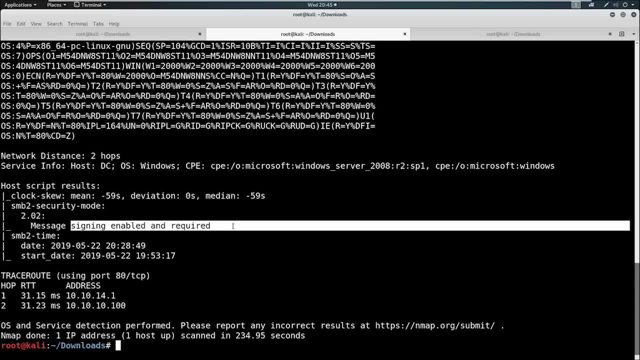 common to domain controllers. smb signing is enabled and required. most of the smb relay or the ntlm relay is done other than domain controllers. sometimes you're lucky and it's turned off. but microsoft got smart and enabled that for windows server. i don't even know what. 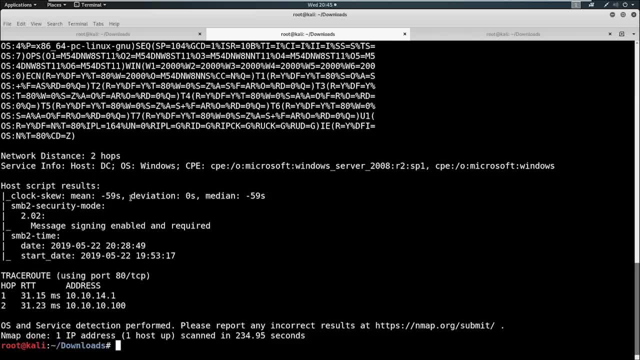 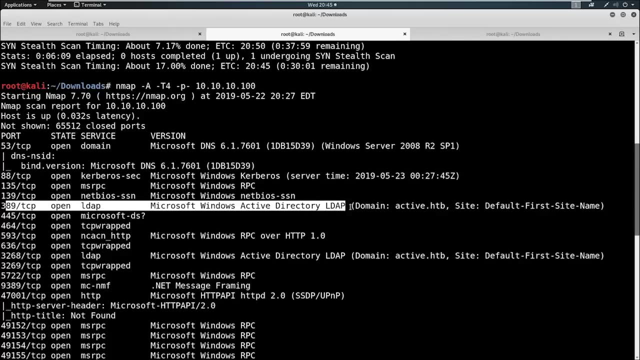 versions onward, but it's, as of late, been running this just fine, so this looks like 2008, so god knows how long it's been doing that. um, and other things that we could look at. right, if we, we can maybe dump ldap information that's a little bit more advanced and outside of the scope. 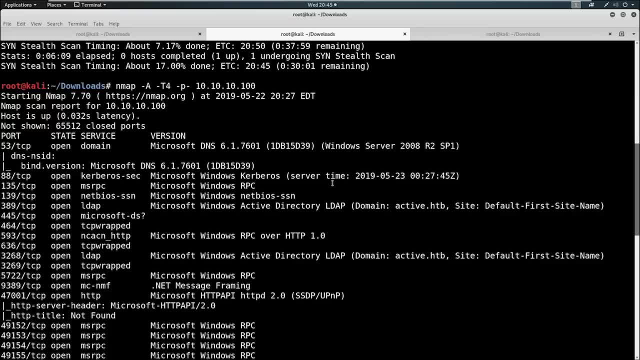 i've seen that done in some hack the box without credentials, but typically you're not going to have access to that without credentials. um, but that's something to to think about and to study, like if you get this box back on an assessment and say, for example, it's the only box. 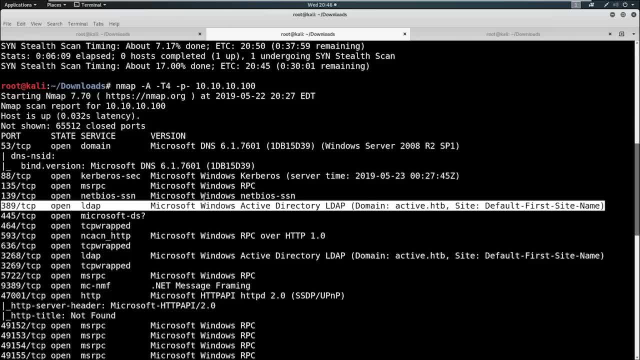 you're going to want to look through each single one of these ports and say what's interesting to me, right? uh, the first thing that's always interesting, and in my behalf, is always 445 and 139, because the more time you spend in pen testing, the more time you have to realize that smb is. 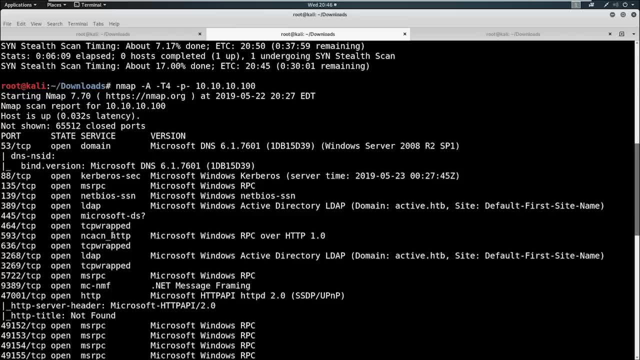 behind a ton of exploits. um, so do note that. uh, it looks like they may have some sort of htp api going on. uh, i would investigate everything that says it's open and probably not tcp wrapped, so definitely worth looking into. so here, first thing we're going, 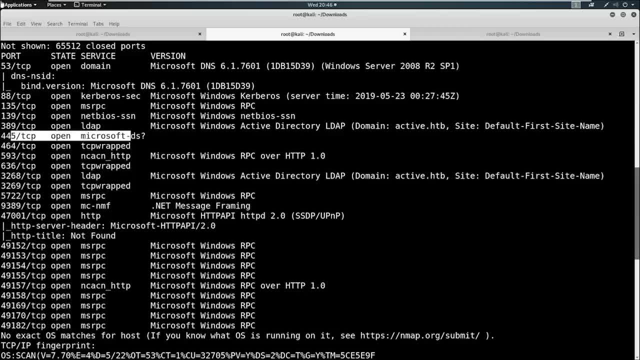 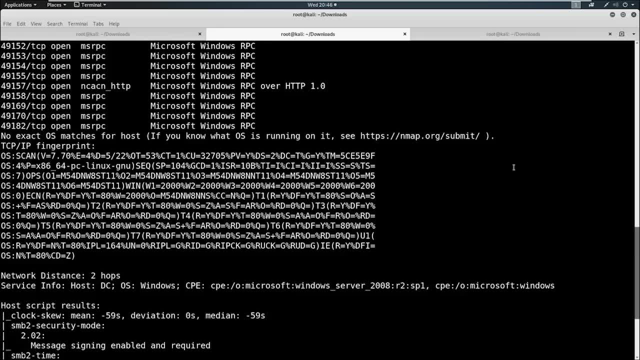 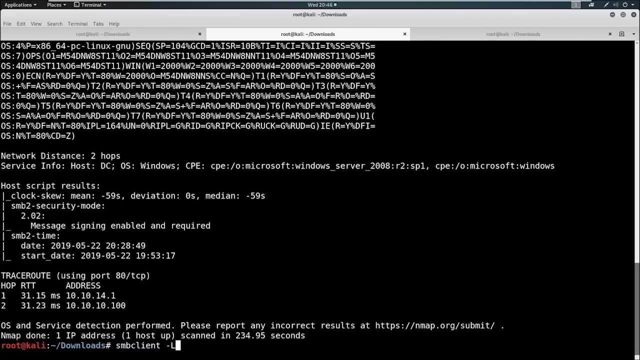 to look into is going to be 445. so what we're going to do is i'm going to go in and use a tool called smb client. so it's going to look something like this: we're just going to say smb client. we're going to do dash l- i think it stands for list. don't ask. 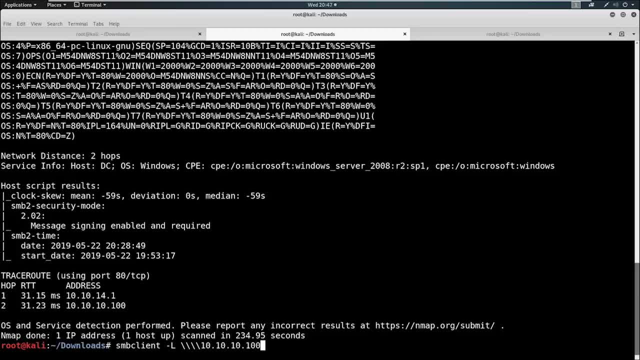 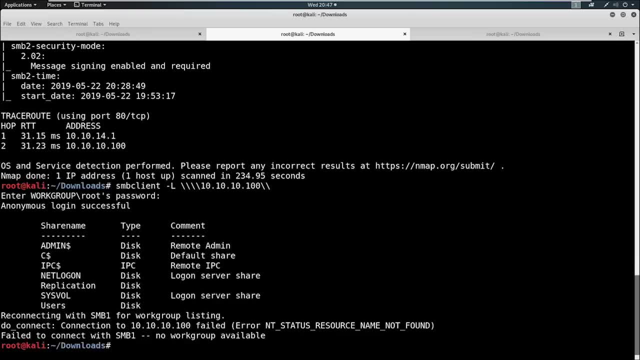 me what it stands for. i don't really know, and we're going to list out the contents of the directory. it's going to ask for a password. we're going to try hitting enter and it says: anonymous login successful. this is a finding, uh, so this finding is that we shouldn't have anonymous login, right? you shouldn't know what sort of 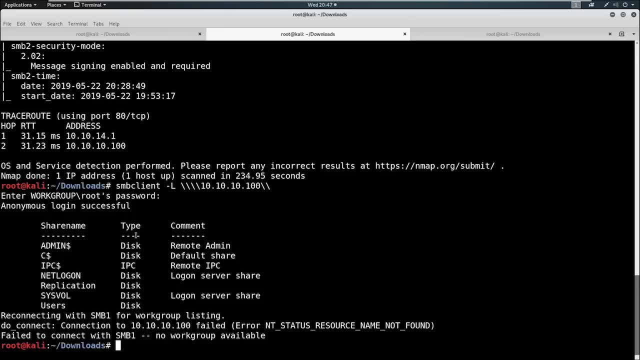 smb shares are out there, so we've got these, these shares here. we're able to see those. we would absolutely list this on our report. now, what we can do with these shares depends on how critical you know this finding becomes. right now it's just a low finding. 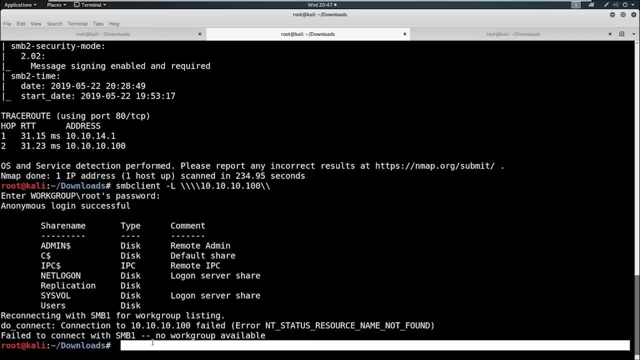 close up the anonymous login. so from here, we'd want to see what folders we can actually connect to. now. the juiciest folders might be something like the c share or the remote app or something like that. so we're going to go ahead and see if we can connect to the c share or the remote admin. we can see if we can connect to those. 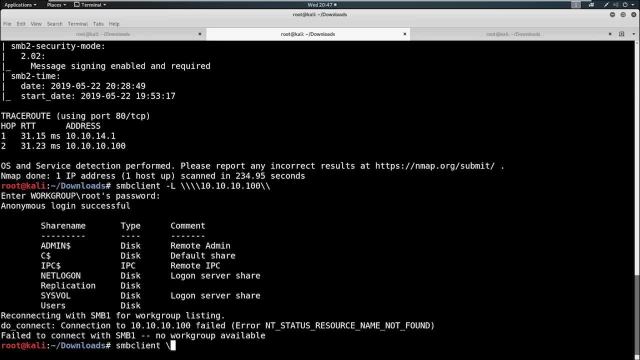 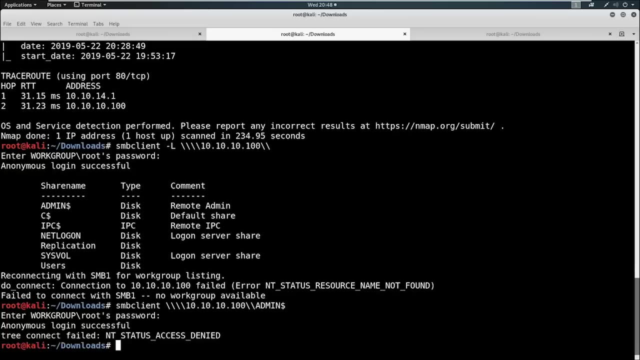 folders. so to connect to a folder, we just say smb client, we do the character escaping, just like i'm doing here, and we'll just say something like admin: dollar sign and try to connect, hit enter and then says access denied, even though we have anonymous login successful. 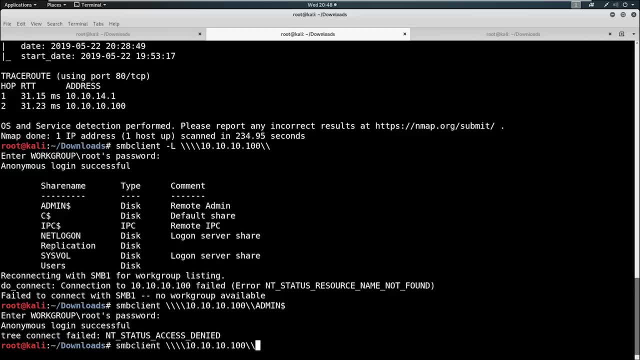 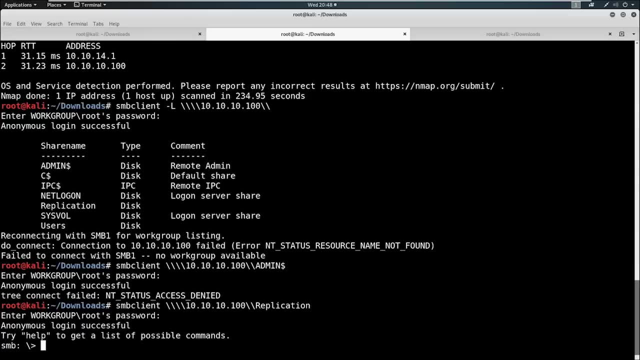 so i'm gonna cheat a little bit and tell you that the one that works here is the replication folder. so we're going to hit enter. we hit enter, enter again. we are successful. okay, so we have an smb login here. we are in this replication folder. now, if we type help, we could see a full list. 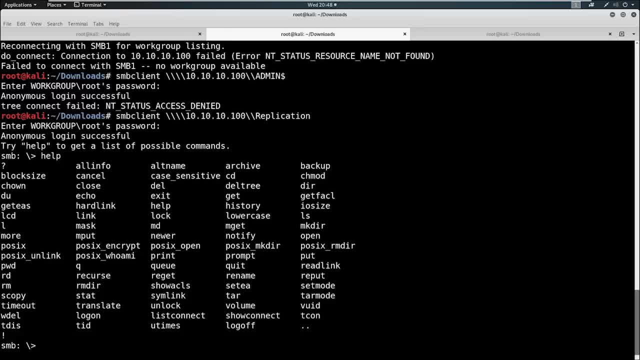 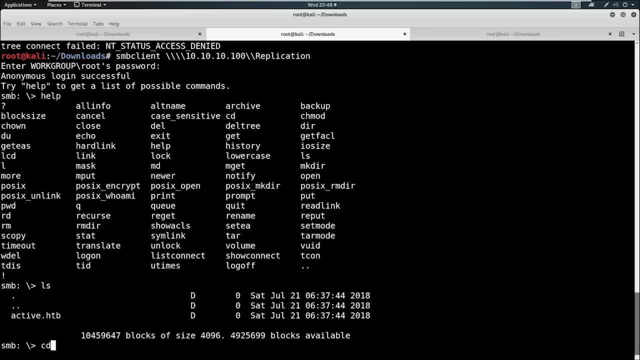 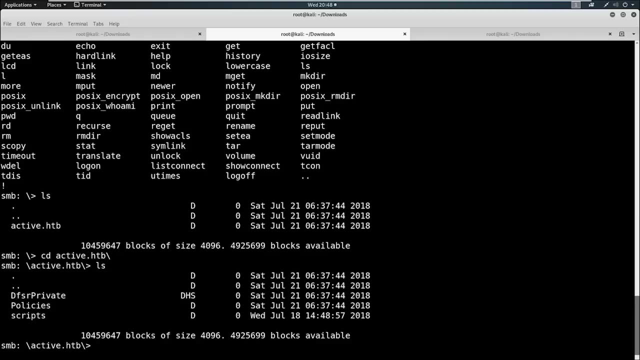 of commands, of what we can do. it's very, very similar to linux. we can say ls and see what's in here. okay, it looks like there's a folder called activehtb. we could say cd, activehtb, ls again, okay, policies, scripts, dfsr, private, and it's called replication. so it looks like it's probably a. 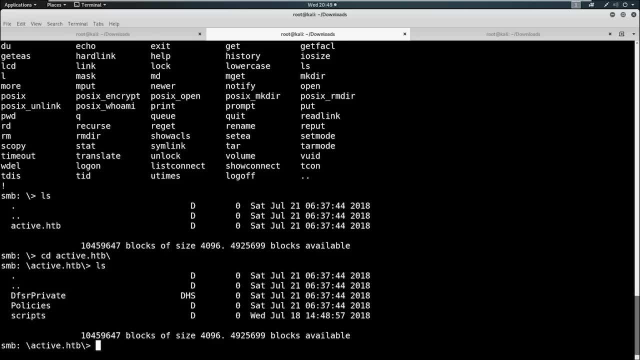 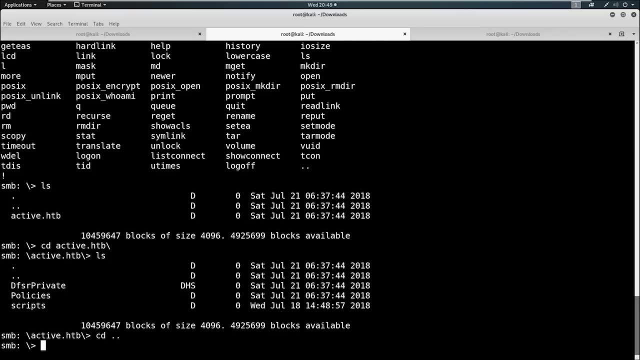 backup of something, right, uh, and a backup of what who knows? but we can figure that out for ourselves. let's cd back a share instead of digging through all these files. there's an easier way to do this. so let's just say we want to download all the files and folders that are here. 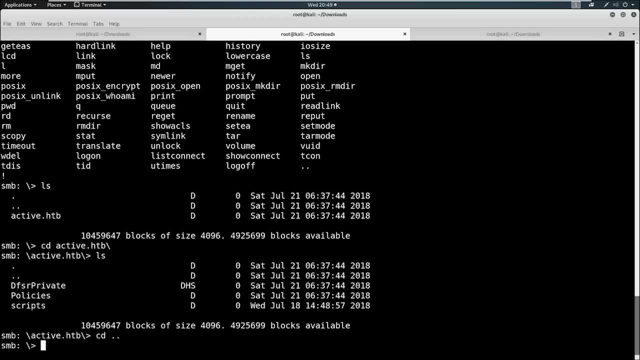 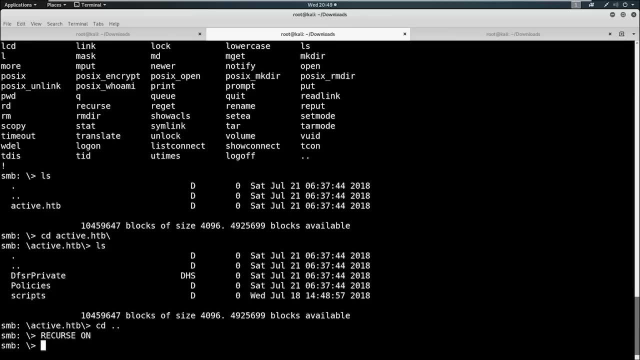 well, we're going to want to do that. we're going to want to do something called m get. but before we just do an m get, we're going to say recurse on, because we want to download all the folders recursively and to save some time. we're. 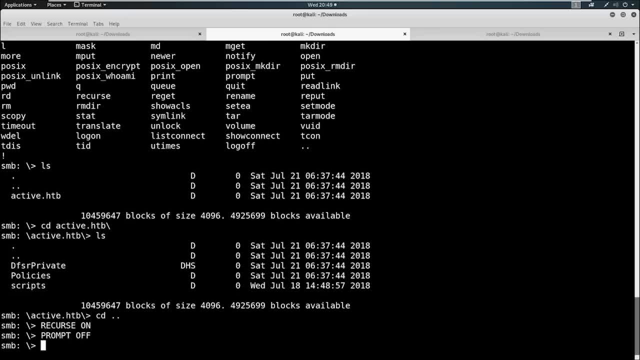 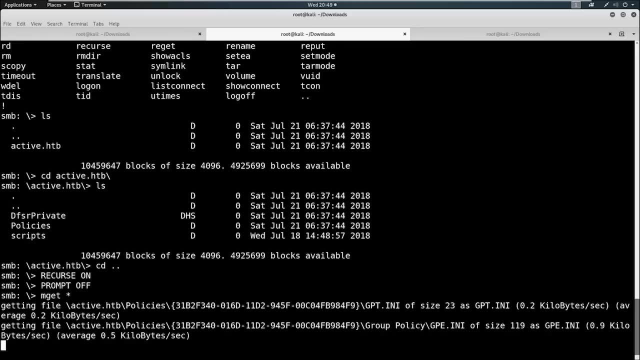 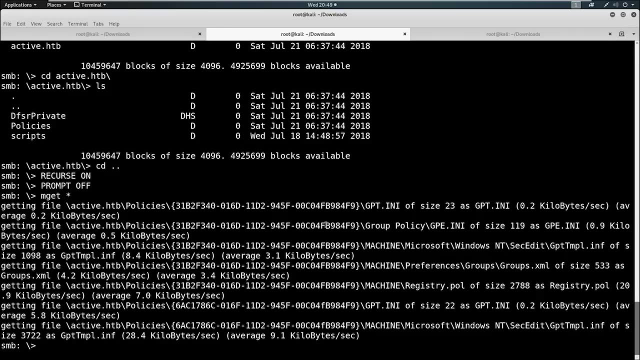 just going to turn off prompts. so we're just going to say prompt off and now all we have to say is m get with an asterisk like this and it's going to start downloading stuff. okay, and we only grabbed like eight files here. if we look through the files that we're grabbing, looks like we grabbed gptini. 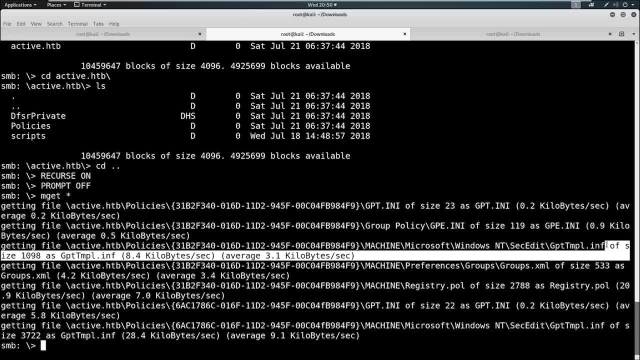 gpeini, a dot inf file, um. and then i see, okay, i see this groupsxml. this is something that is really well known to me, um, and this is something that is likely going to be pay dirt for us. so let's explore what's in the groupsxml and then we'll talk about. 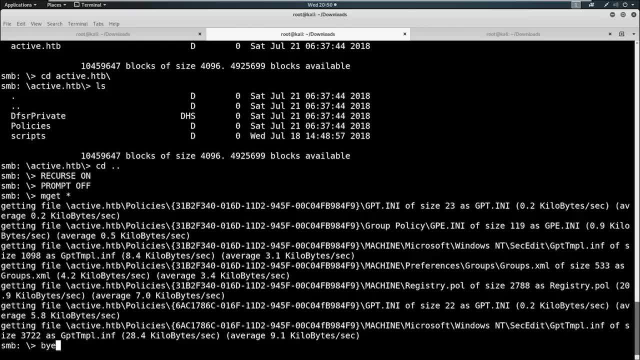 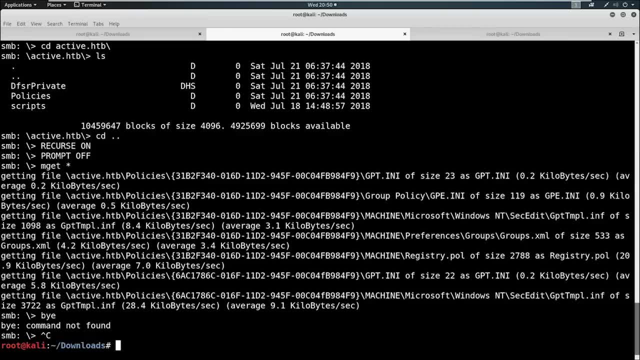 what's in the groupsxml and then we'll talk about why it's so relevant. so i'm just going to say buy. okay, i guess there's no buy here. uh, just ctrl c. if we ls in this folder or we say um, cd, i think should just be active. it should have the same folder structure. so we say: 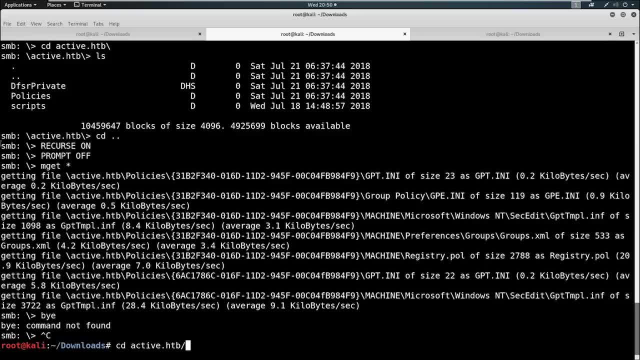 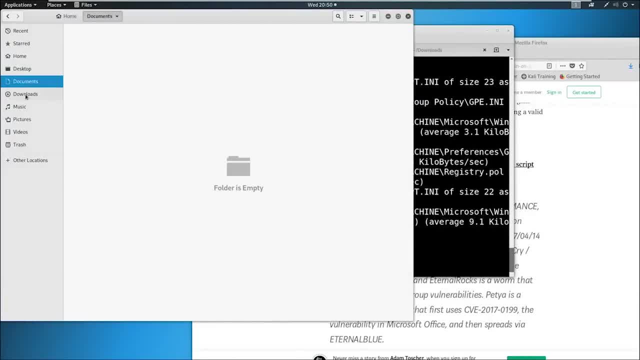 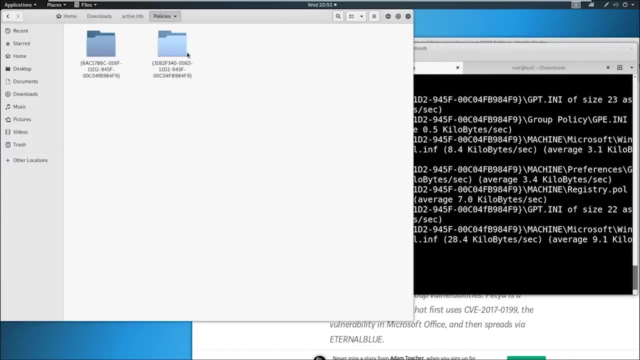 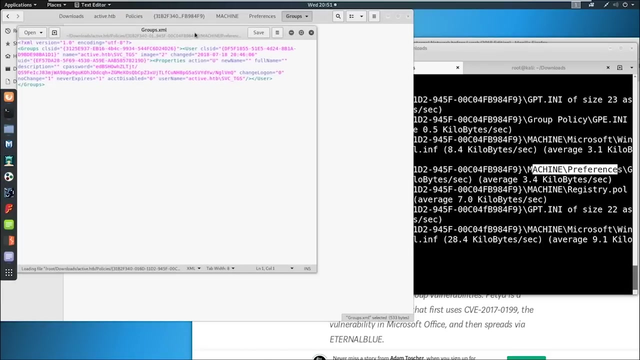 active policies. uh, actually this would probably be better to just do in a gui form: documents downloads active and we say: um, it was policies. policies 3: 1 b, machine preferences groups, and we open up this groupsxml. okay, so it might be a little hard to see. 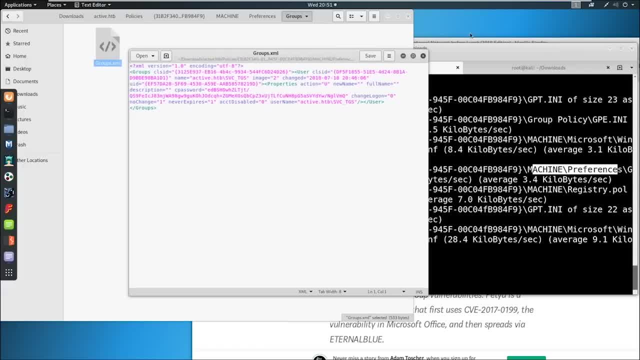 so let's talk about what this gpp is. um, this groupsxml is. so groupsxml is related to something called gpp. uh, it's also group policy. preferences is what it stands for. an easy way to remember this on a pen test, if you ever listen to rap. 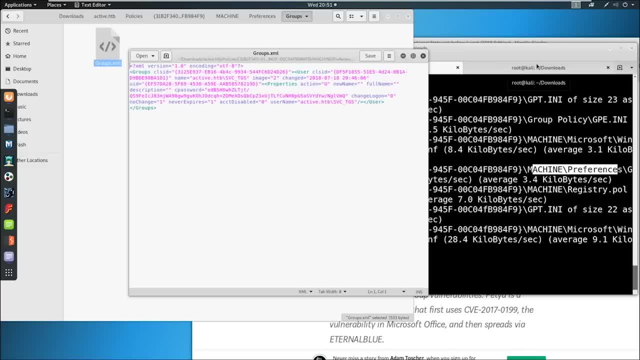 uh, there's a song called: are you down with opp? well, just think to yourself: are you down with gpp? and make sure that you search for gpp, right? so you've got this group policy preferences. and what it did was it allowed domain admins to create domain policies using embedded credentials? right, so the credentials are. 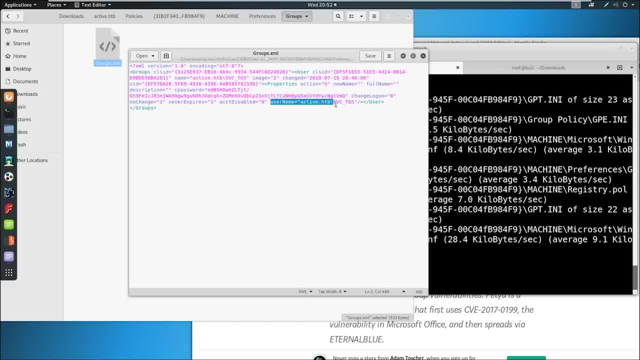 right here in this file you see username, activehtb. and then we've got services tgs here, this ticket granting service- and we'll talk about the ticket granting services here in a second- and then you see this thing called the c password. this is what we're after, and there's actually a great article by rapid7. 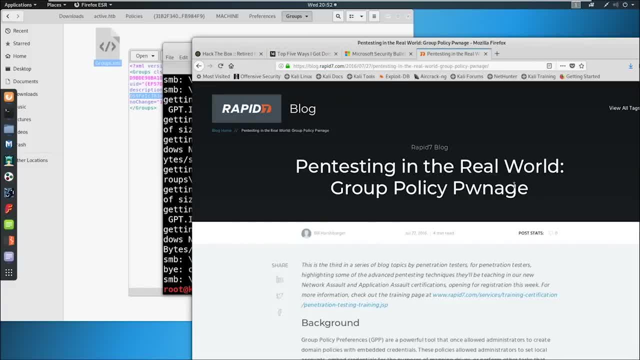 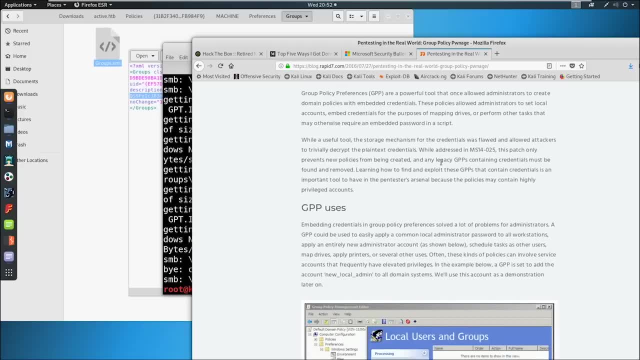 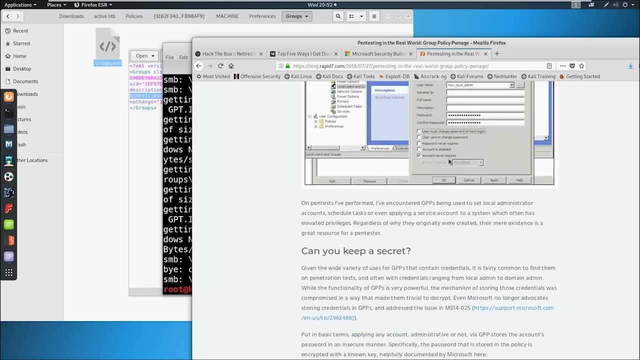 that i've got up here. it's called pen testing, the real world group policy pwnage. it talks a little bit about gpp and what it does. uh, probably better than words i could put it into, but basically you were able to store the uh username password and you created it right for for an account to do some. 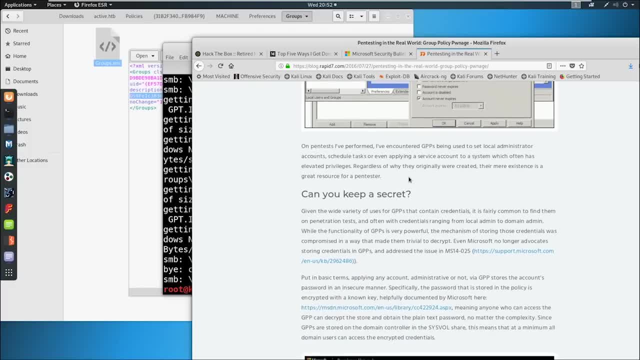 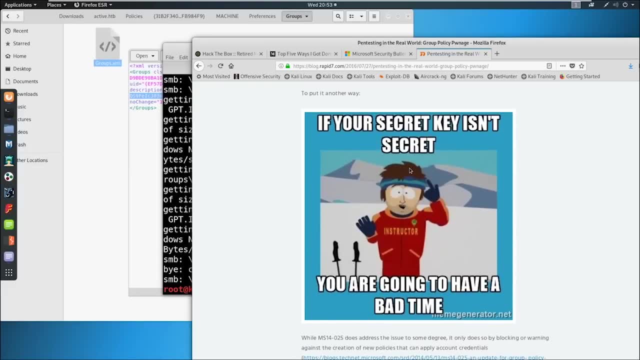 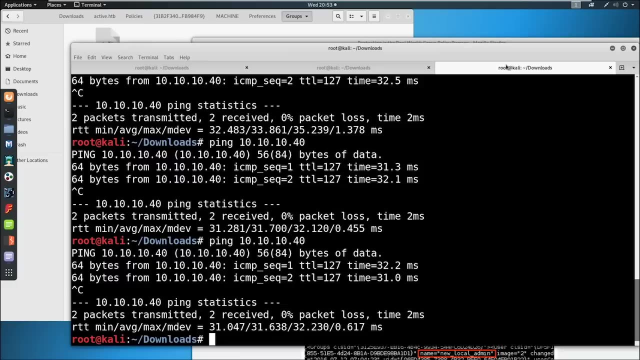 sort of action and say file sharing or whatever it is, through group policy. uh, this was up until a few years ago. so these keys just stored in this sysvol folder, right, and what you can do is there is actually a metasploit module which i want to show you. we won't use it tonight because we 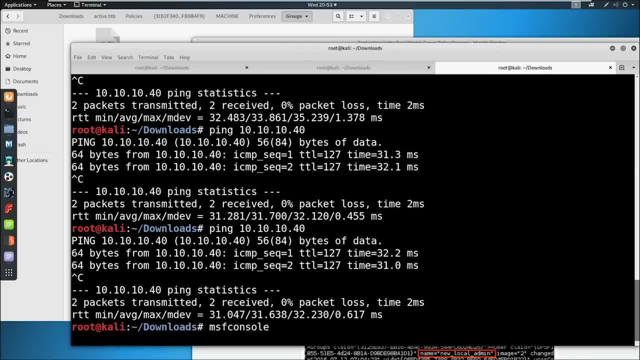 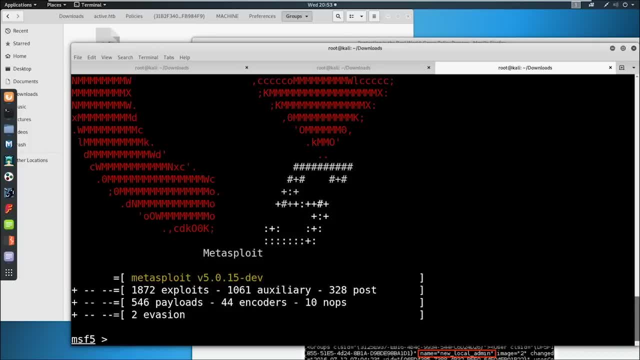 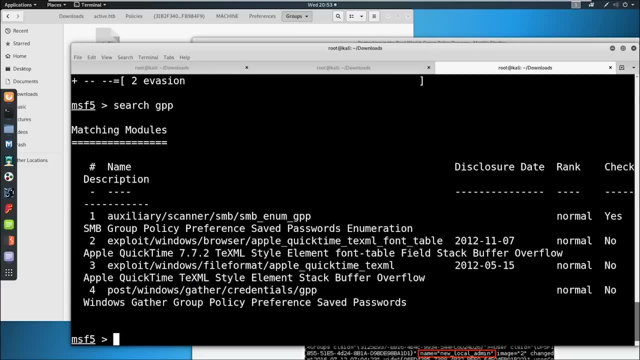 have no need, we've already got the file. but i run this on every single internal assessment and you believe how many times the C password or the GPP, it just shows right up. So if you search GPP, does the groupsxml file exists on an active domain? it exists on some active domains. 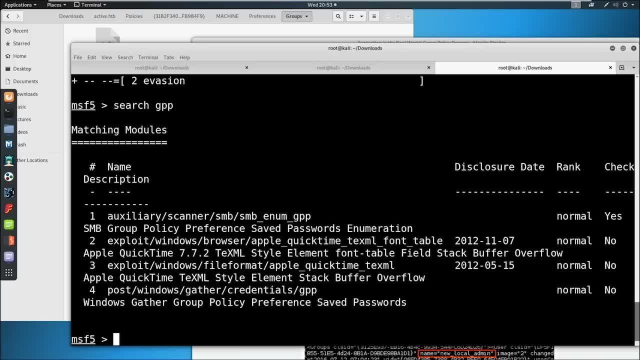 this is for older domains, But sometimes, even when they migrate, they leave that file in there And we're going to talk about that too. So if you see the post, windows gather credentials. so as long as we have some sort of access on a session, we could say: use post. 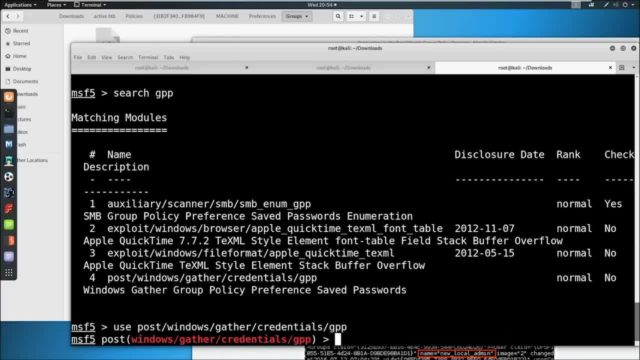 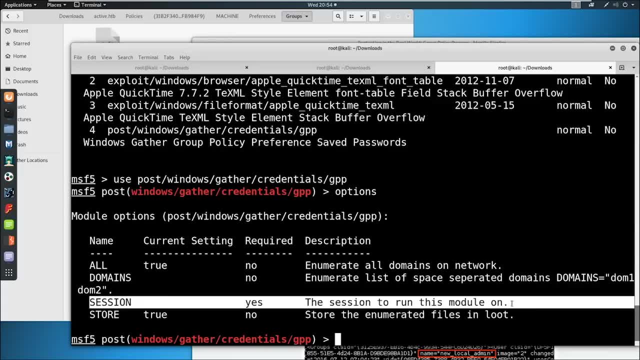 windows gather credentials: GPP. look at the options. So we need a session, right, It could be a PS exec, whatever session we get. Once we have a session, we can run this. we may be able to get the a domain administrator password just from this, So very, very important to try to run this. 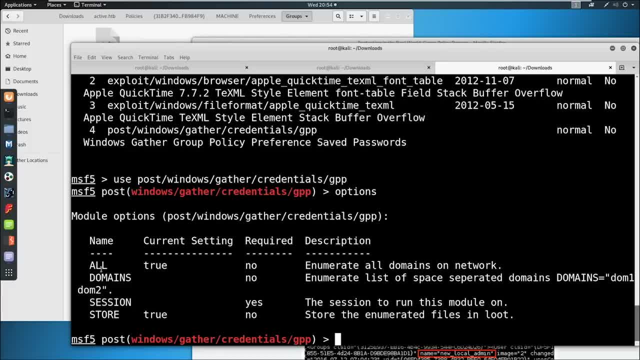 on any any internal assessment that you can. So another thing to note, though: we have set this up in the past for clients as what's called a canary account. Basically, what we're doing is we put in an account that has a GPP or C password, and it's never been used, But 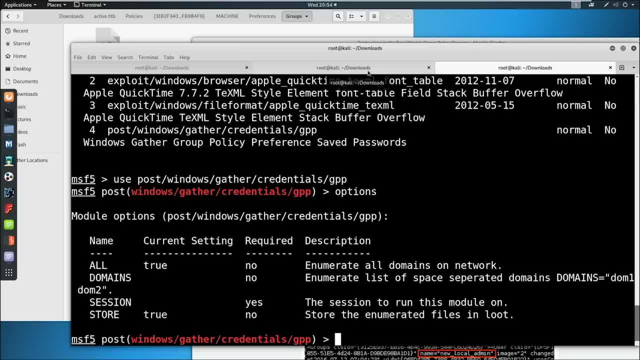 we're basically sitting there as a honeypot, right? So when an attacker is in your network and they're looking for this low hanging fruit- because GPP is low hanging fruit- we say okay, they find the file, they see the username credentials And as soon as those, 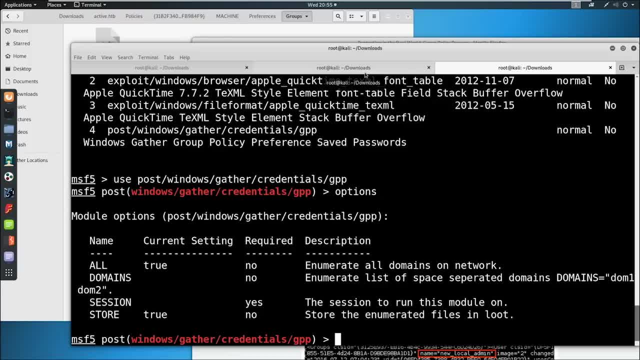 username credentials get activated, then we know an attacker's on the network, right? So just because this is low hanging fruit, your competition might be using it as bait, So always think about that as well. But typically on pendants you're going to see the same thing, Like I'm gonna put. 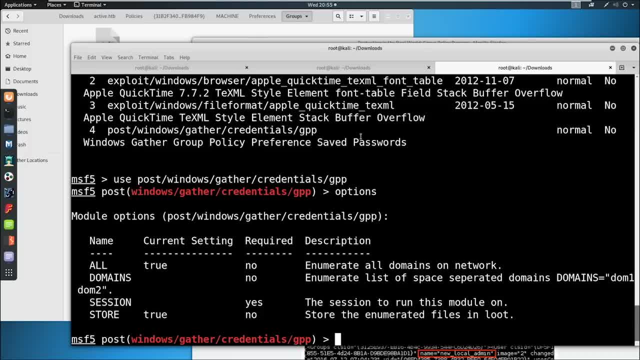 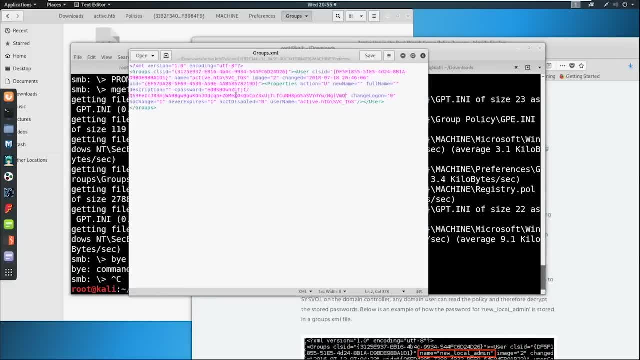 typically on pen tests. it's something that we'd grab right away. Okay, so let's talk about how we can exploit what we just found. So let's open up this file. we've got the C password here. I want you guys, if you're following along, to copy the C password, And what we're going to do is say: 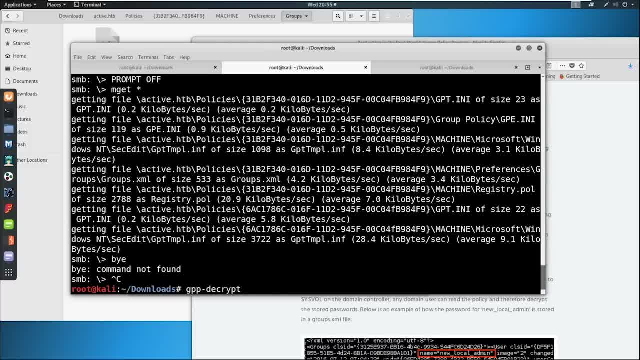 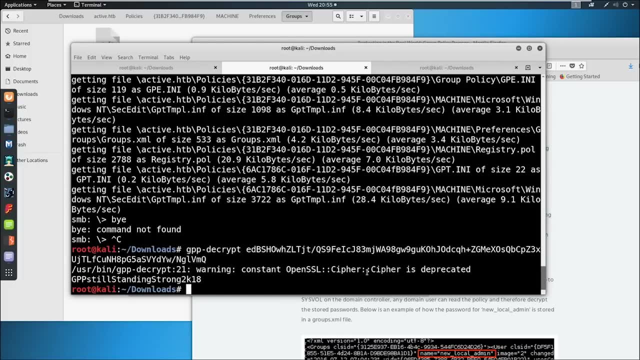 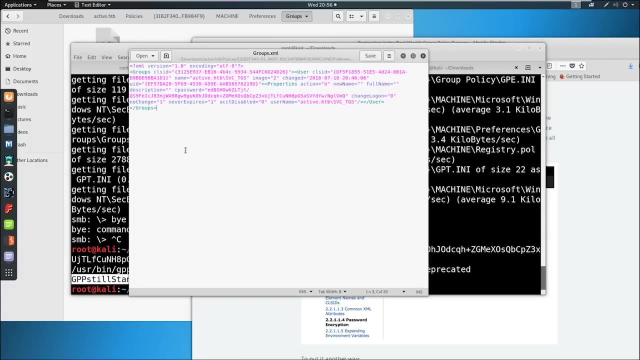 GPP decrypt. it's built into Kali And then we should just be able to paste this password here. We get a warning, but don't worry about it. the ciphers deprecated. So what we're going to do is we're just going to copy this And we are going to. let's just paste it somewhere that we can have it. 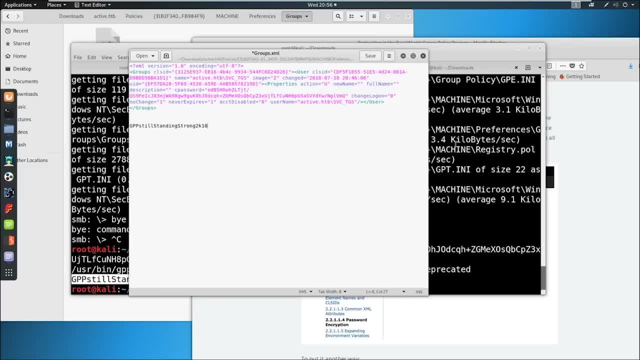 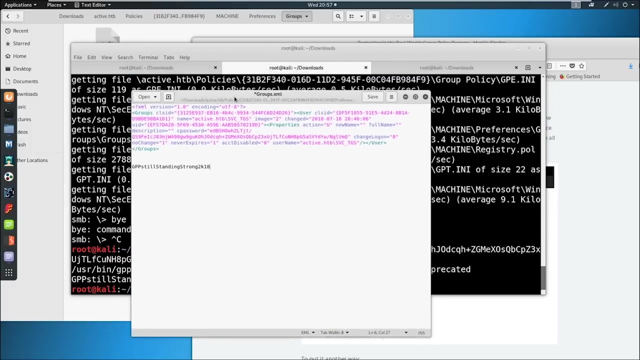 right, Okay, okay. so what this means now is we have a account, we've got this domain here active, dot htb. we've got this service ticket granting service account here. So what can we do with this? Well, we can use again crack map exec. try to push it around. 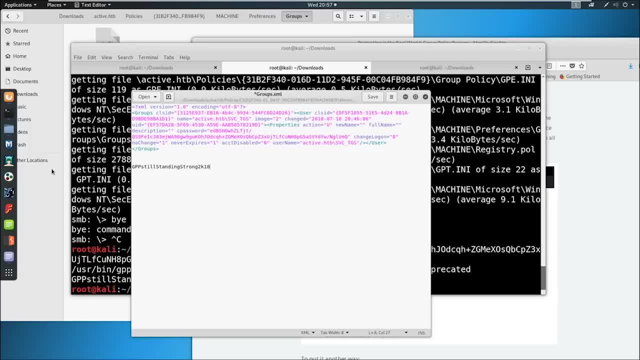 right, See, see what we can do With it. we can try to go back into the SMB client. try to login with this account. see if we can get into the admin folder. You know I could use PS exec on this machine. That was the first thing I. 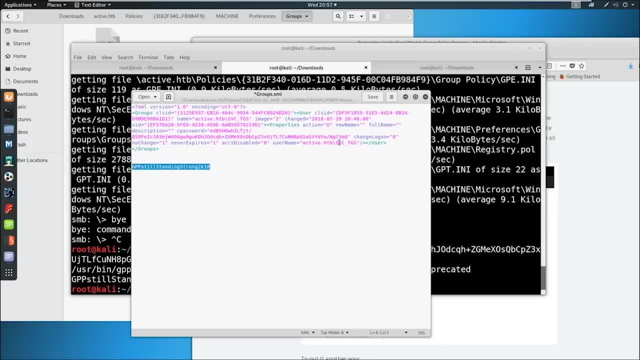 tried when I did active was to say: okay, does this have access to, to the share folder and administrative privilege? So I tried PS exec. PS exec doesn't work either, but be thinking about the same process for everything you're doing. So PS exec. you know crack map exec, exec, so you can. 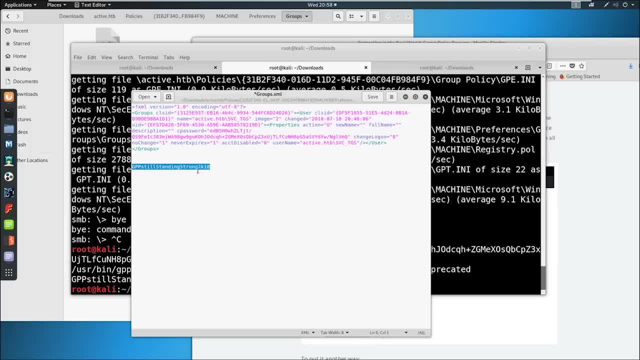 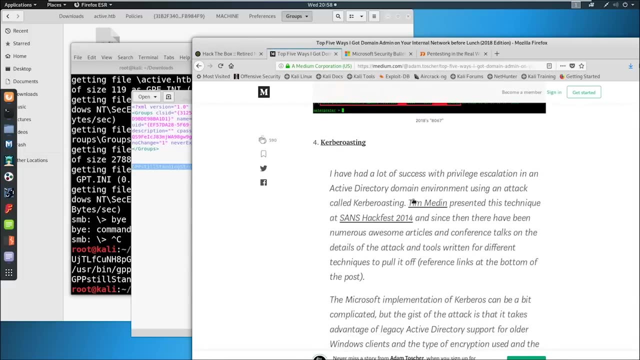 etc. Whatever we can do with these credentials, we're going to try to get in anywhere and everywhere that we can. Well, we're in a one box network right now. So another tactic that we're going to talk about, and tactic number four on this list, is Kerberosting. So we are going to 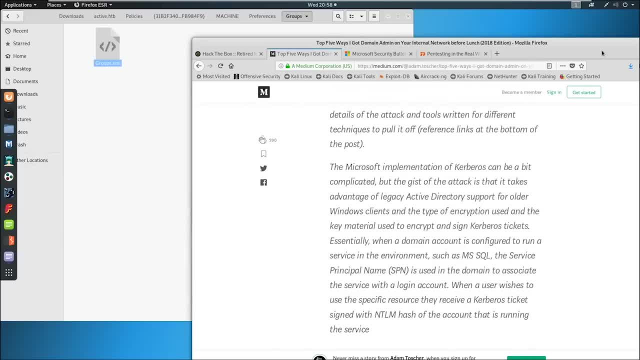 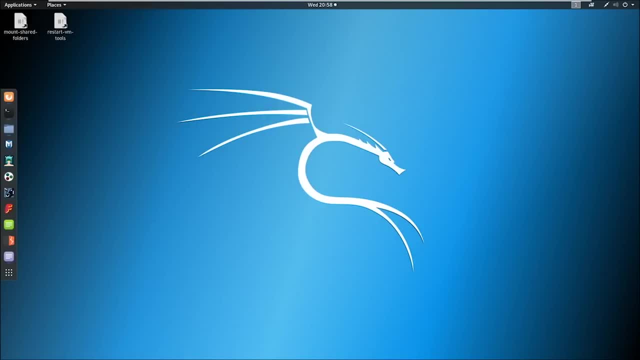 talk Kerberosting. Let me minimize everything and bring out my handy dandy pen, And so I can explain this as best as I can. There's probably going to be somebody out there who is a domain guru and going to correct me on this, because you people like to correct me all. 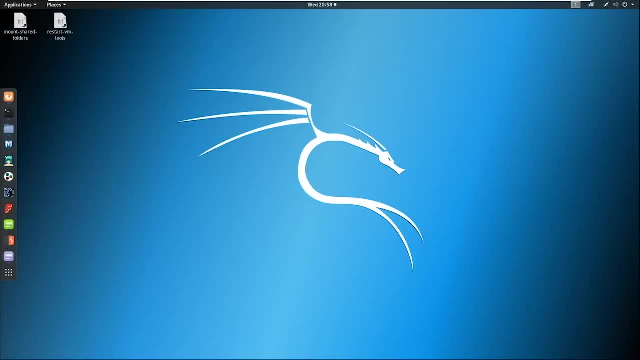 the time when I say something wrong. So sorry in advance if I, if I miss misquote this Right. So let's talk about my best interpretation of what Kerberosting is And before we can do that, let's talk about Kerberos. So Kerberos is just an authentication. 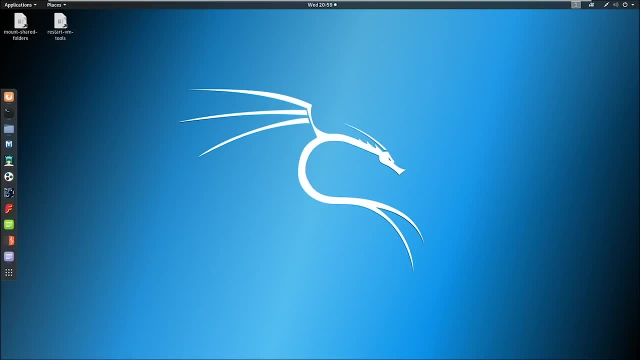 protocol. right, It uses tickets. So it's using tickets as a form of communication and authentication. So let's assume a situation and this is how it typically is. That is a huge fucking thing. All right, Let's clear that. Let's try that again. All right, We've got this machine. 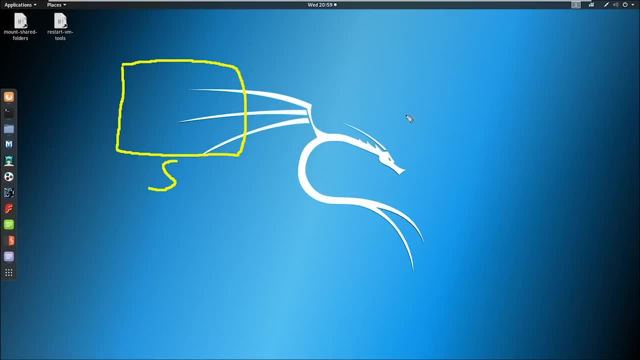 here. This is our server. Our server is also considered a KDC Right. It's a key distribution center because we're giving out keys. All right, We also have another computer here. We'll just call that the client Right. 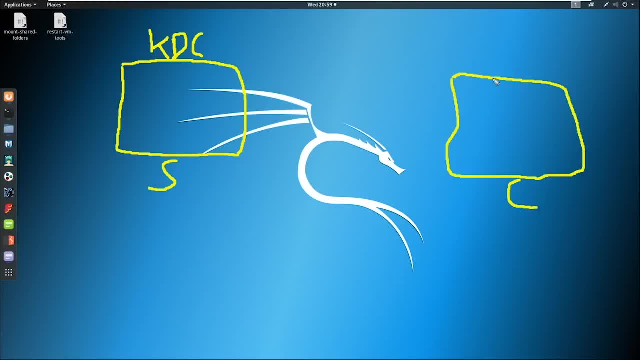 So we've got the client and the server. Well, let's say the server or the client wants to authenticate, Right. So it's going to come to the server and it's going to say: hey, server, you got those tickets. Can I get a ticket? It's going to ask for a TGT. 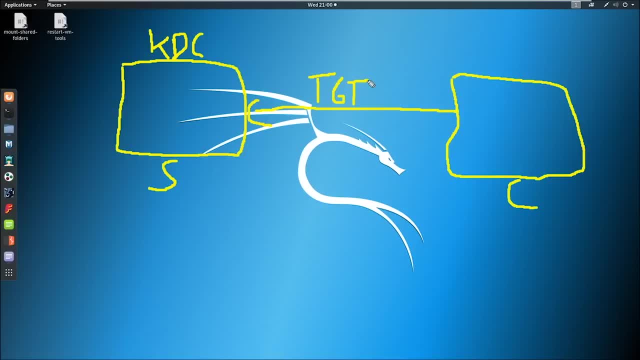 a ticket granting ticket. Now the server is going to check the credentials and if the credentials are good, it's going to send back over encryption, which is called TGS. Ticket granting service is going to encrypt a secret key. Remember key distribution center. It's. 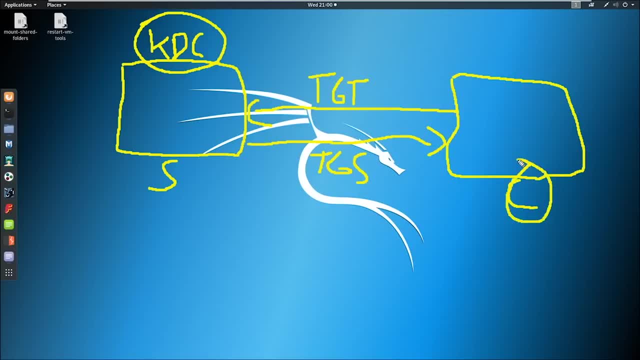 going to send back a secret key that gets stored on the client. So this client has a ticket. It's stored here until the ticket expires. Now let's add upon to this story. Let's say that there is a service that we want to connect to Right. Come down here. We'll just call this. 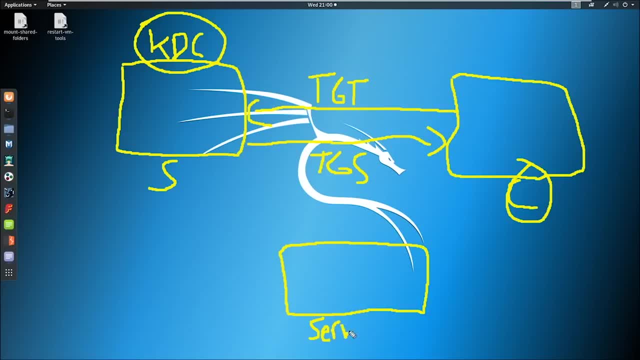 service. And a service can be whatever we want, can be SQL, can be antivirus, you name it, But let's just call this a SQL service. OK, Services have what we call SPNs. These are service principal names. So to connect as a client we need to ask for permission to. 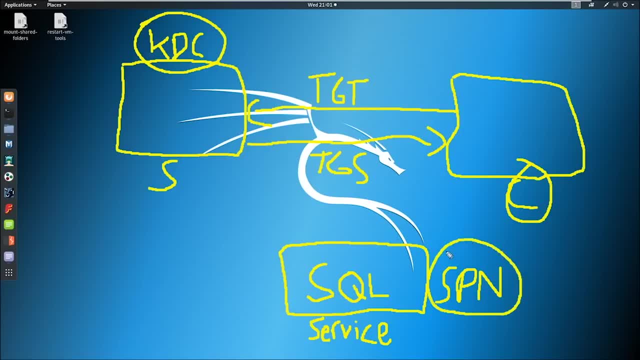 connect to the service We need to know. We say, hey, the SPN, I've got my ticket, I'm going to take this And can I? can I please connect to this SQL service And we get a session key back from? 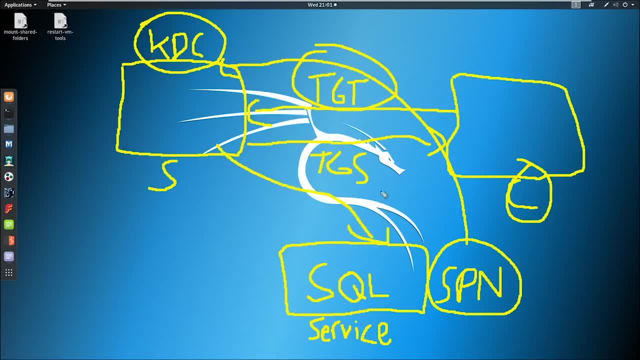 the server if we have the credentials right, or the ticket at least, to connect. So the thing to know about Kerberos is that it's going to send back a secret key So we're going to connect to. is that with any valid ticket or TGT we can request for a TGS ticket for this SPN? 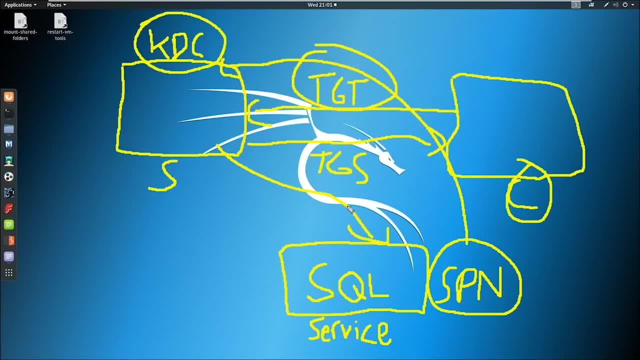 So lots of acronyms, Right? If you're a military, former military, you're probably following along just fine. But there is a lot of little letters here. Just know that if we have a valid ticket, we can request via the SPN, here at least to attempt to get a TGS Right. So we're going to 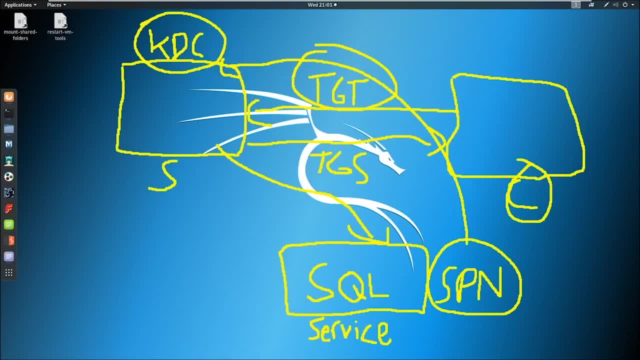 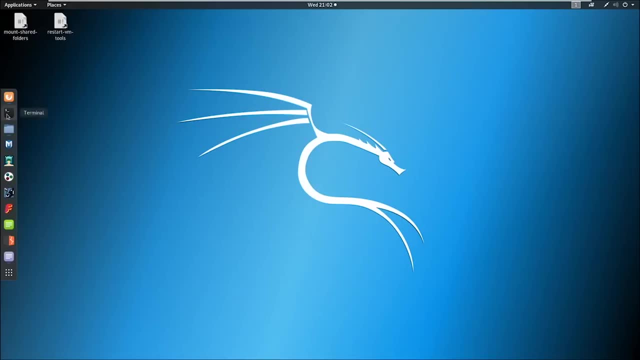 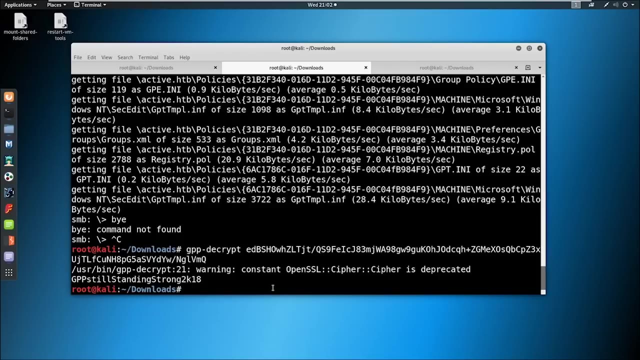 see what that looks like. There's actually a tool that does that. It does that for us. How did I do you domain people Did I do? OK, All right, let's pull this back up, And this is part of the impact it. 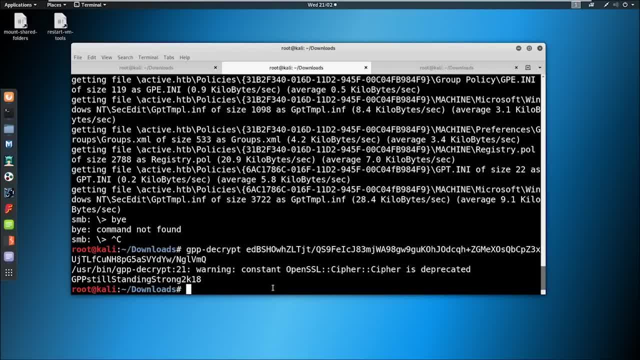 the impact. it right, The whole thing we've been using this entire time. what we installed in the beginning I told you would be important, This toolkit, So impact, it is awesome. So let's go ahead and locate what we're going to be running. It's called get like a type, get user. 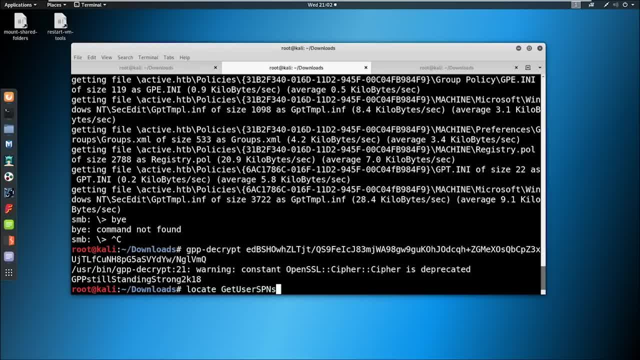 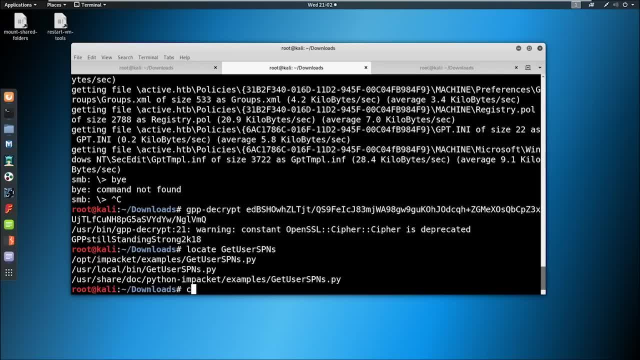 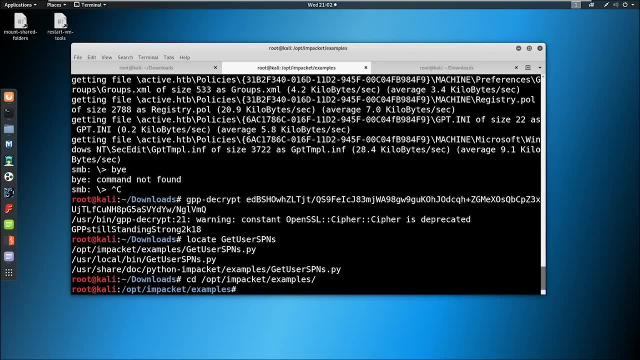 SPNs. You see we have a few. the one we installed them getting the course was the opt impact it. I'm going to use that one. So I'm going to cd to opt impact it examples. All right, So now we ls. there's. 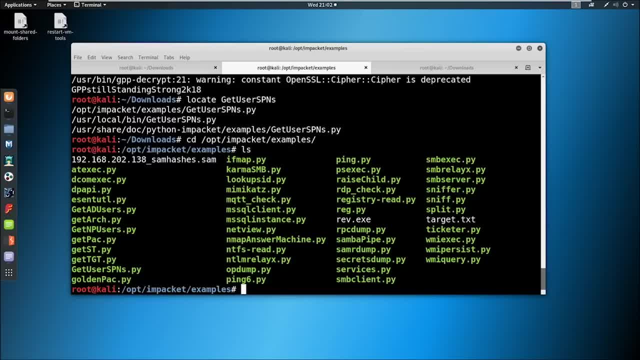 a bunch of stuff in here, but we're going to be using this toolkit, So let's go ahead and locate that. get user SPNs dot pi. We're just going to say Python: Get user SPNs dot pi. All right, First, 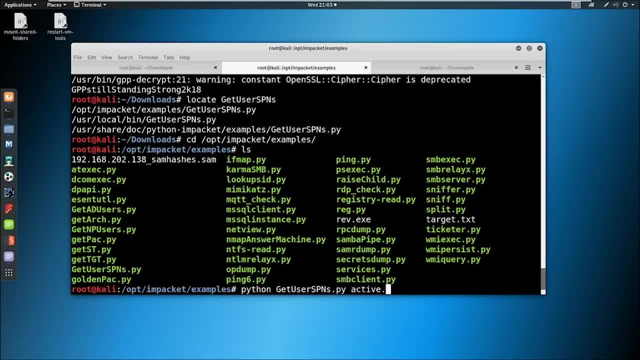 things. first we need the account. The account was active, dot, HTB And it was service ticket granting service right. Next, we need to say DC IP. we need to know the IP of the domain controller. Well, lucky for us, this is the domain controller. 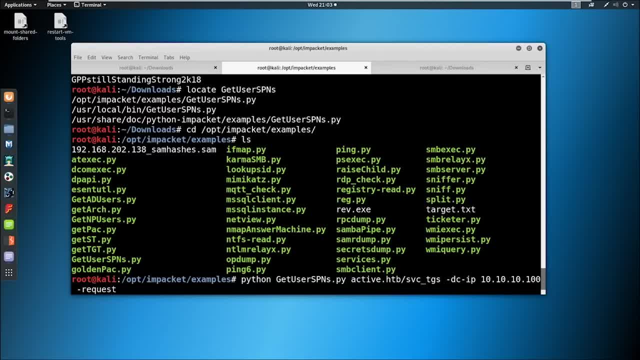 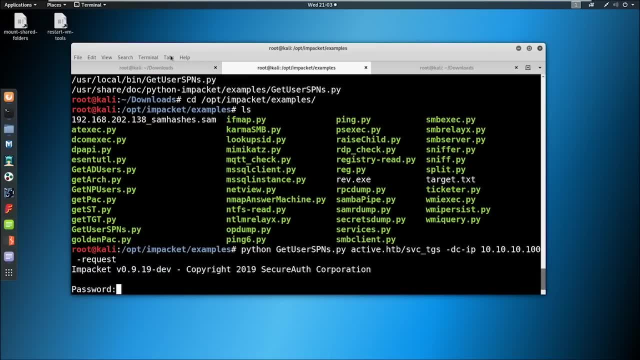 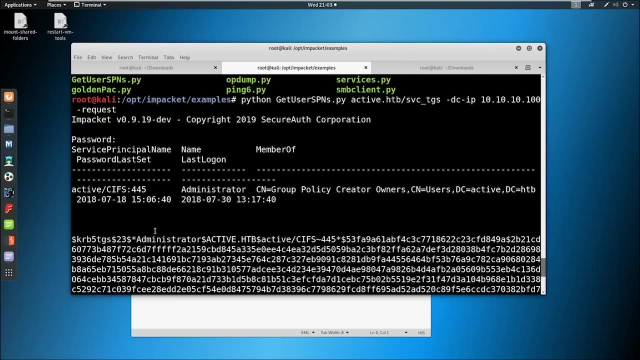 And last, we need to request the ticket. So we're going to request a ticket. Ah, we need a password. So we come back into here, we copy this guy, We paste And we get this wonderful thing back here. So 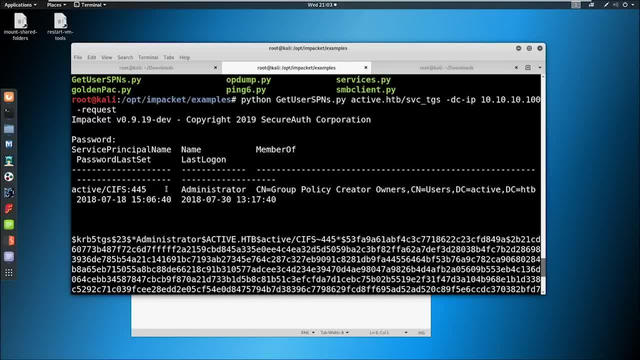 we see that we have captured something here for the administrator right. We've got this long hash And it's a KRB five TJS. So what can we do with this? Well, we can take this offline and try to crack it and see. 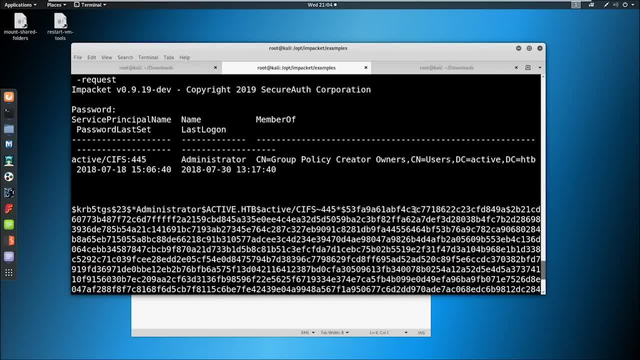 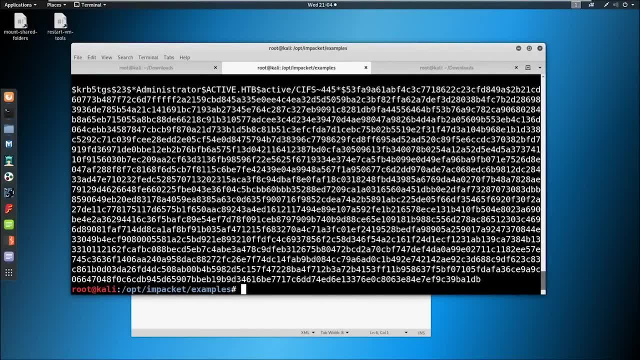 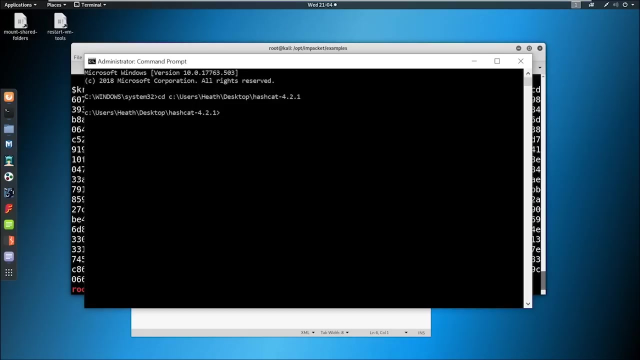 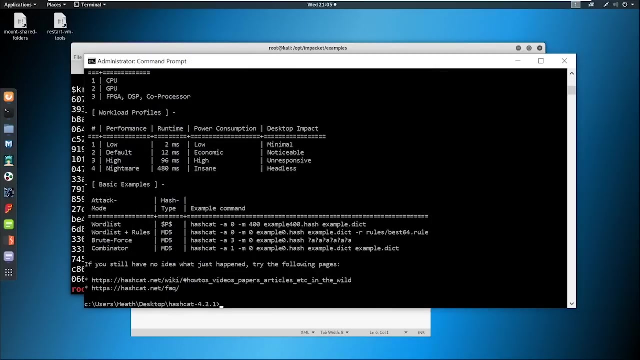 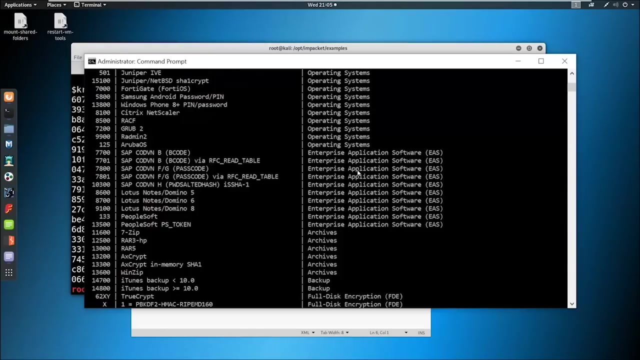 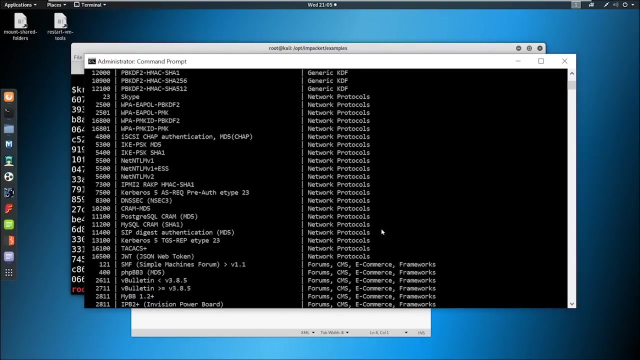 what happens, And we're going to do just that. So have your handy dandy hash cats ready. I'm going to load mine up now. Give me one second. I am not prepared, as you guys are, Okay, So I'm going to run hash cat. We're going to say dash, dash, help. We are looking for KRB five, which is 13100.. If I am not mistaken, Here you go. It's under network protocols 13100: Kerberos five, TJS, TGS, Sorry. 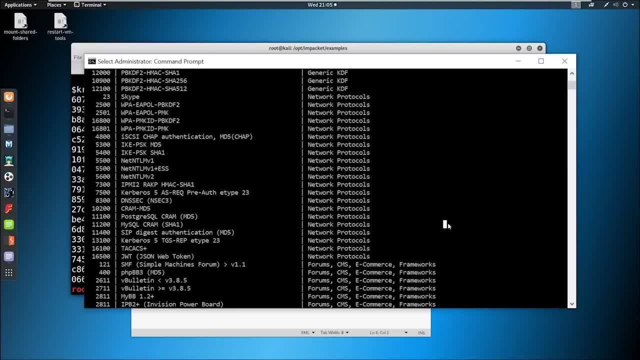 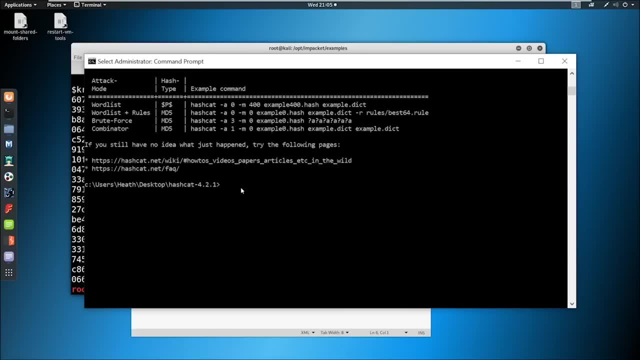 Okay, so we know our module is 13100.. If you've been following on week to week, you should know how to run hash cat now, right, So hash cat 64 dot exe. We're going to do a module of 13100.. I named this file. 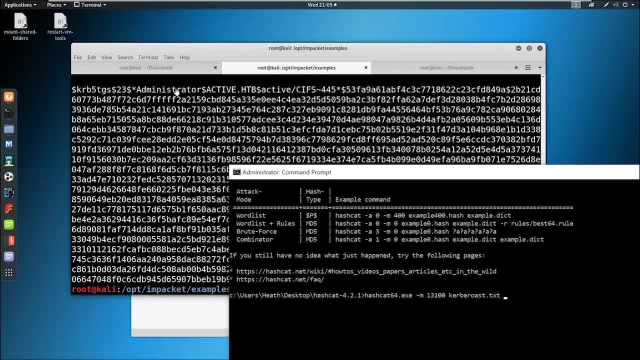 Kerberos dot text And all I did was copy this entire line, all the way down to the end, put it into a file. I'm going to run this whole thing and I might want to submit the answer for it. We're going to definitely do an exactly same file year the next time. 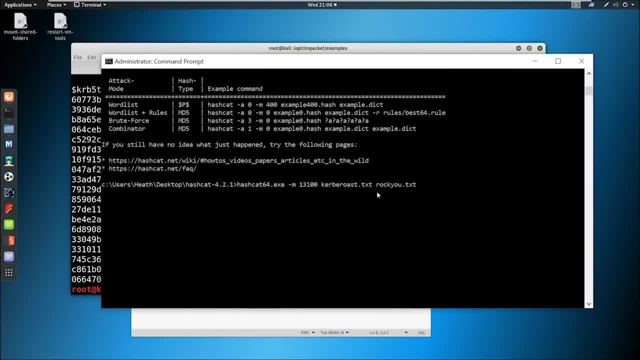 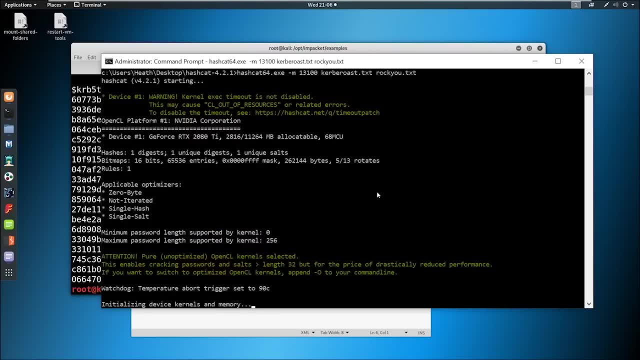 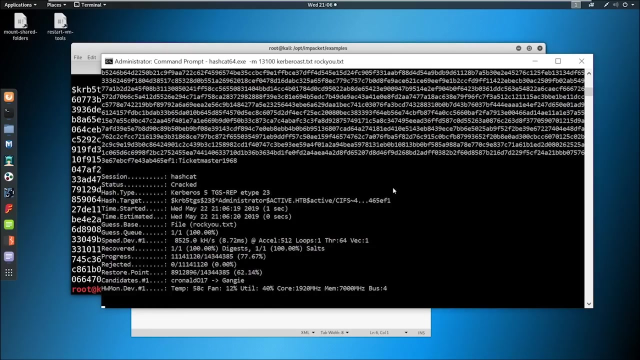 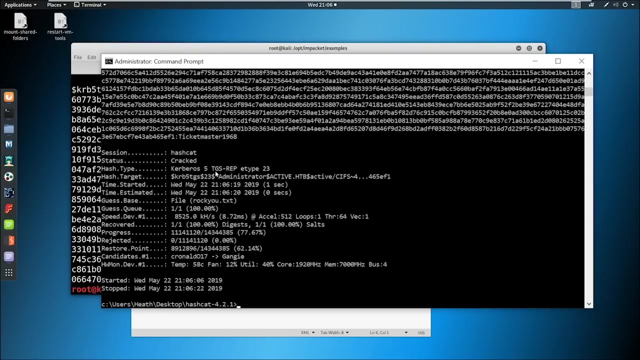 this through rock you. I've got a brand new 2080 ti that we're going to push this through. I haven't actually run any hash cracking on yet, So let's just hit enter and see what happens, And it took us not that long at all, So we went through. where is it? 77% of the. 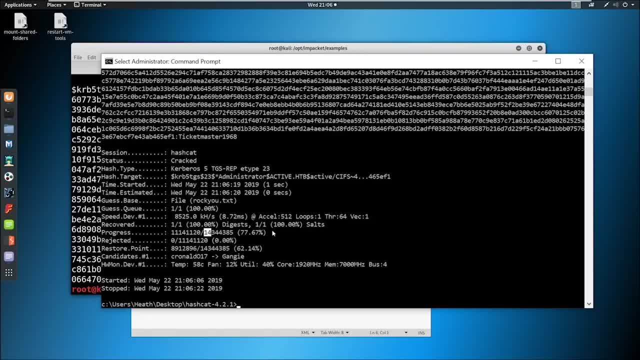 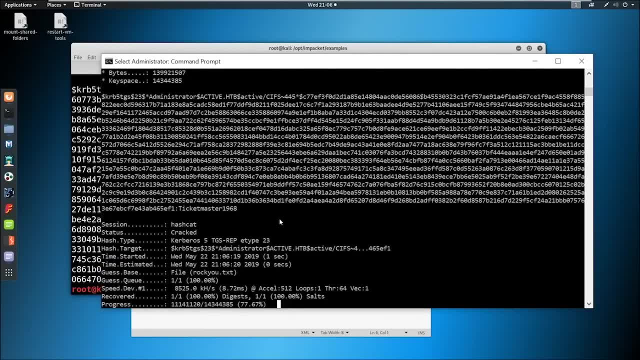 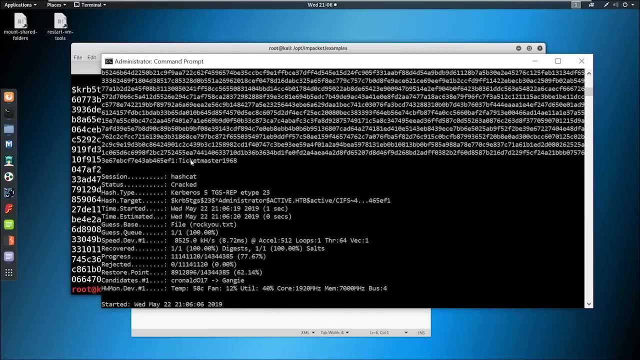 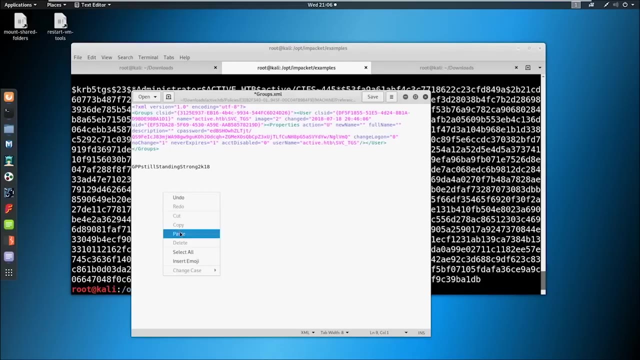 list, and the list is 14 million passwords long. So that's pretty good, All right, so it's cracked. You can see that it's cracked. Ticketmaster 1968 is the credential, So we're gonna take that And I'm going to paste it in here. Okay, And now let's load. 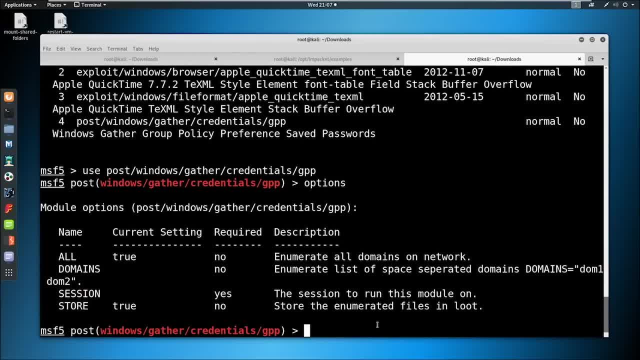 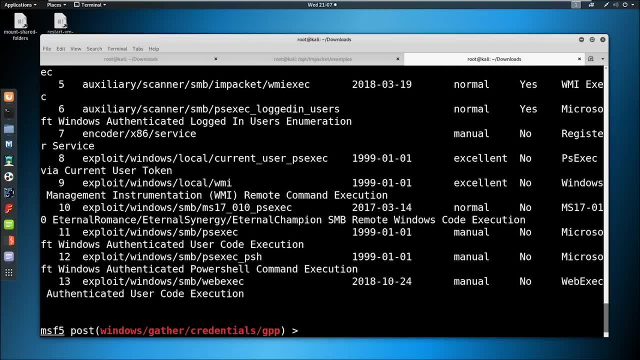 up Metasploit. We actually have it loaded And we're going to do is we're just going to search for PSP, PS exec. We're going to use exploit windows, SMB, PS exec. It's number 11 on my screen If 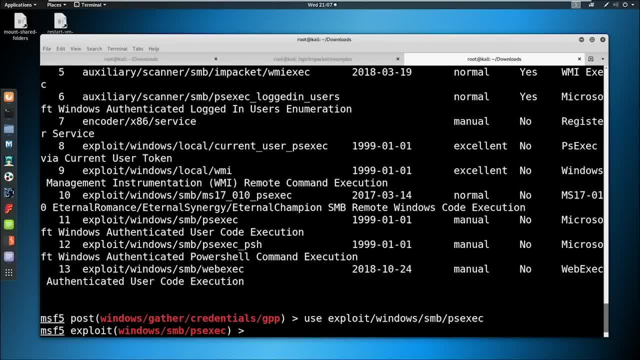 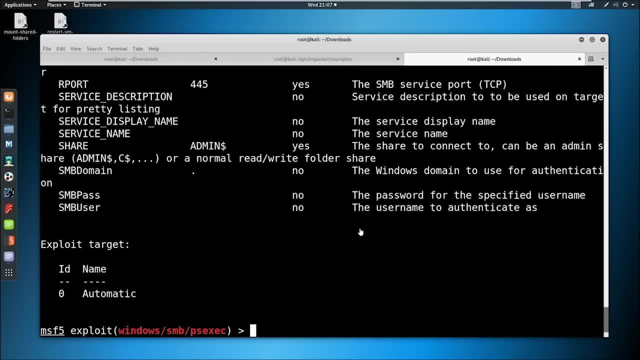 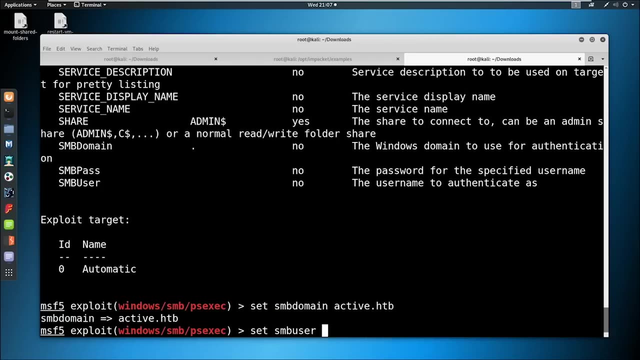 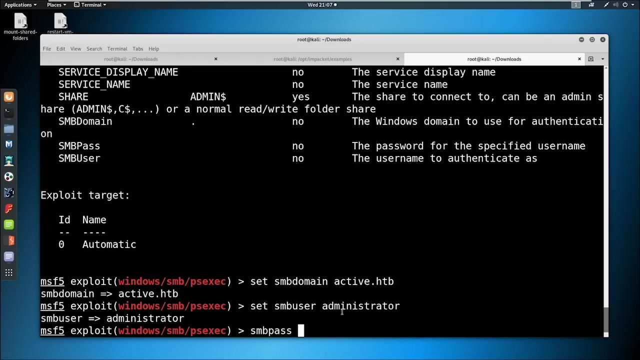 you don't see it, let's talk options. Okay, So we've got SMB domain. Remember that is activehttp. SMB user is administrator. SMB pass: is that Ticketmaster pass, maple 280.. Prinzip 2.0.. 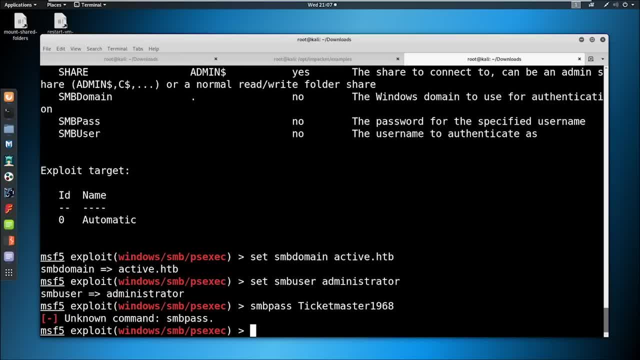 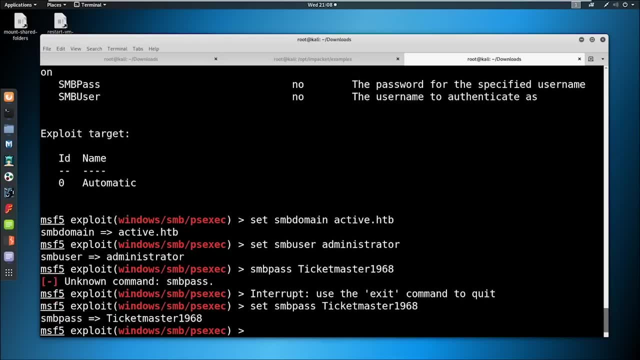 Paine, page 178.. Let's try running it and see if we get lucky. ammed He'sendi. let's try running it, See if we get lucky. I'm kind of indifferent now. Let's run this. Let's see if I can. 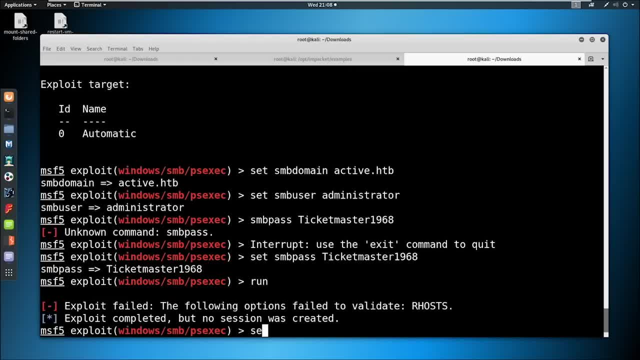 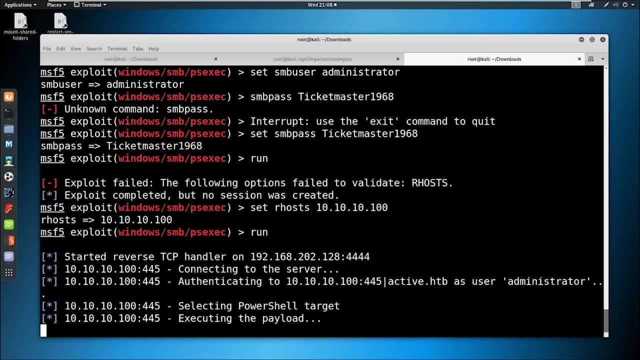 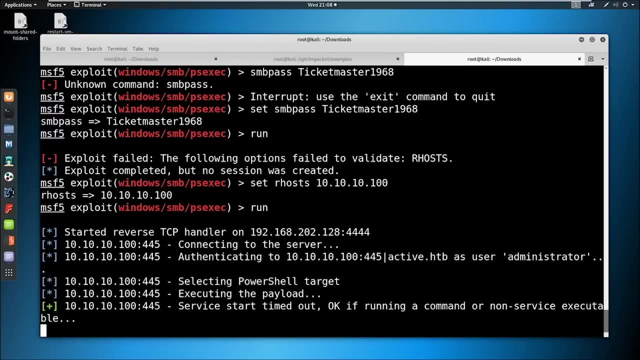 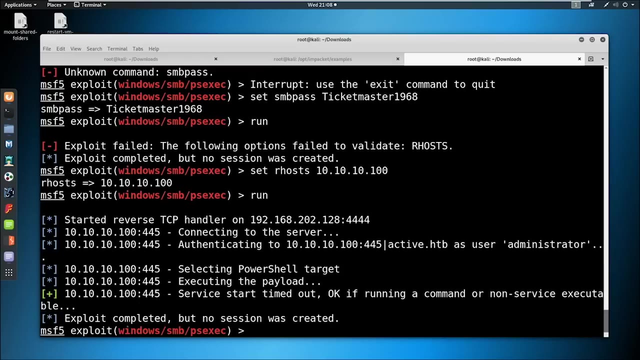 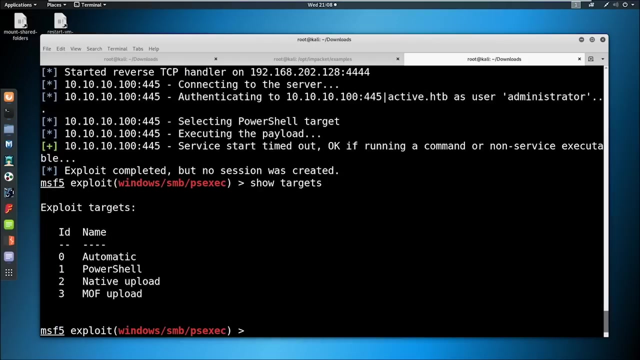 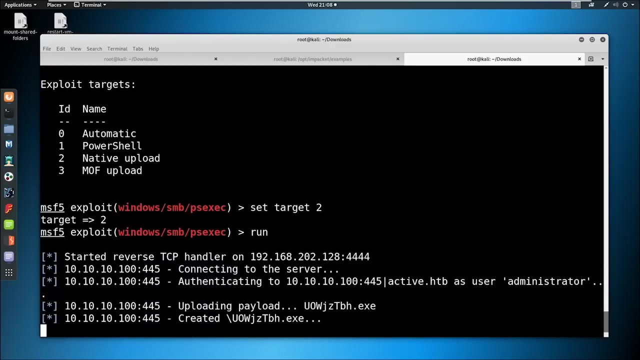 It works. Key. Okay, different on the. I never said in our house. Sorry guys. All right, let's try again, See if we get lucky. Okay, so it's selected PowerShell. Let's look at our targets. So we ran automatic. let's try a native upload instead. 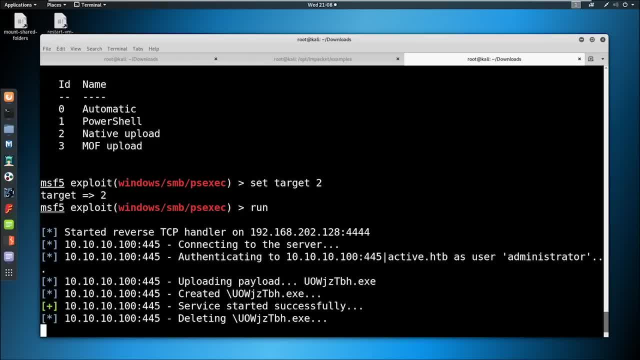 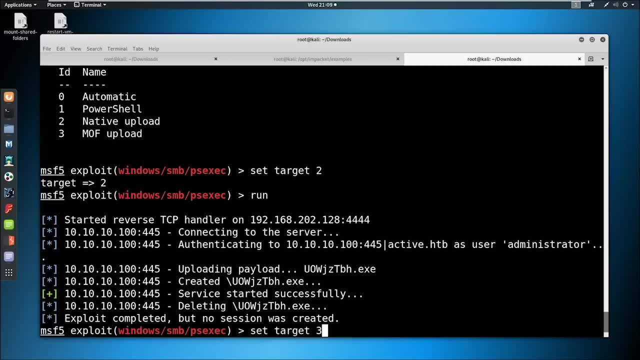 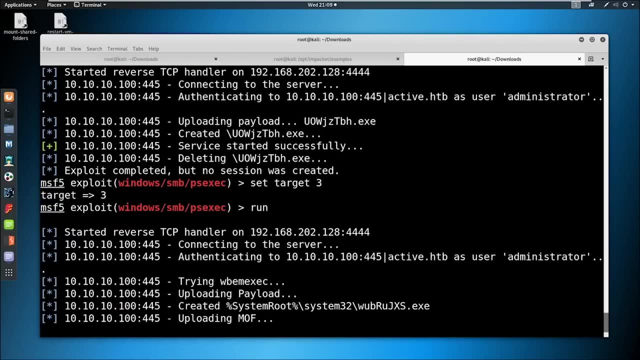 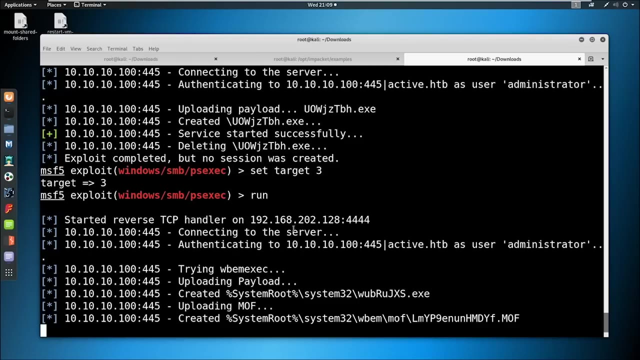 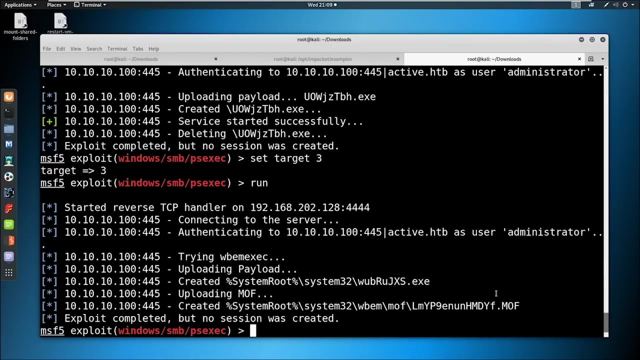 So we see that we authenticated, we uploaded a payload, it's creating, it's deleting And it's hanging. Let's try target three. Might have to go back to target two and pray. Oh, my El host is not good. Good, Good job on that one. 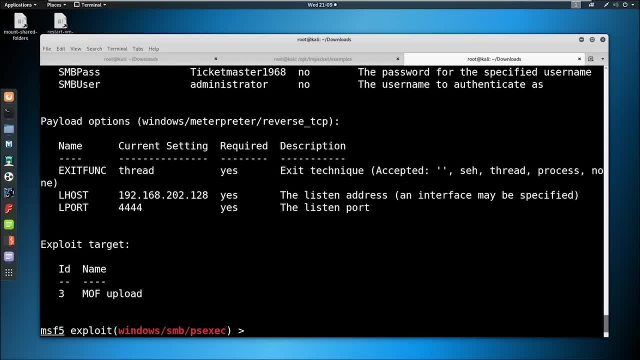 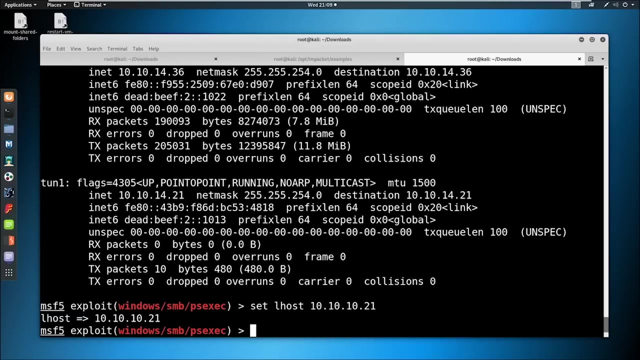 So, as pointed out, thank you very much. The El host got pointed to my machine and not not the Cali machine or the, the IP address that's here. So let's set the El host. If yours did that, also set yours. I think mine's 36, Oh no, it's 21 now. 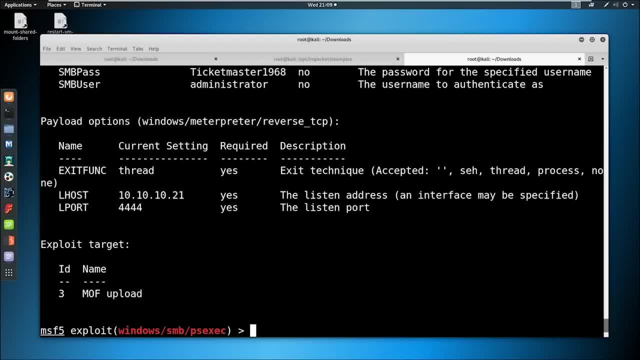 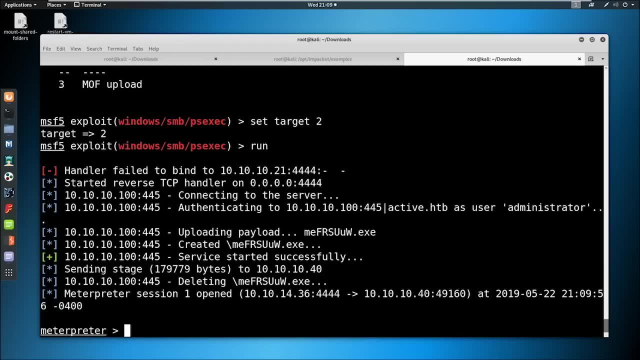 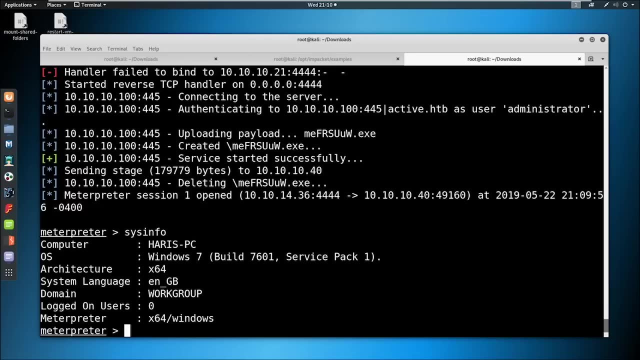 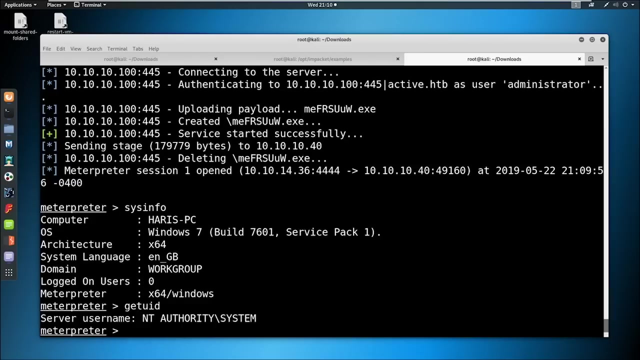 All right, So set target back to two and run again. There we go. Thank you, techno bro. All right, so we've got a shell sysinfo on the shell. 64 bit meterpreter, 64 bit architecture. Get the UID. We are authority system. we have full access on this PC. Again same concept. 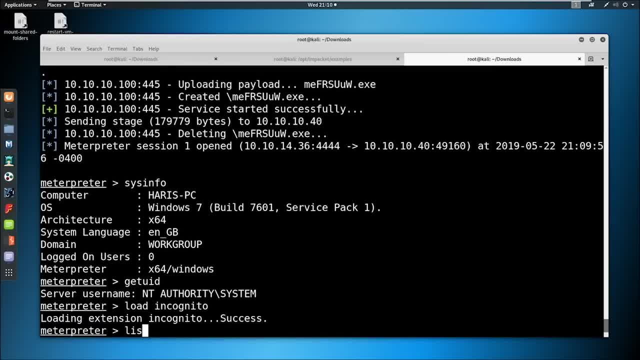 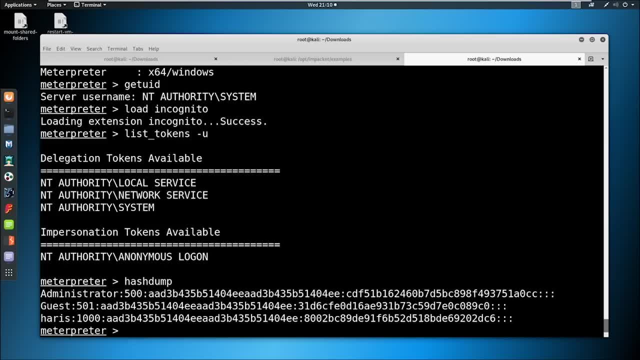 here, right, We would load incognito list tokens see what tokens are out there. we would do a hash dump: dump the hashes, pass them around, see what information we can get from that. This is one of the more realistic boxes, like I said, in terms of you know. 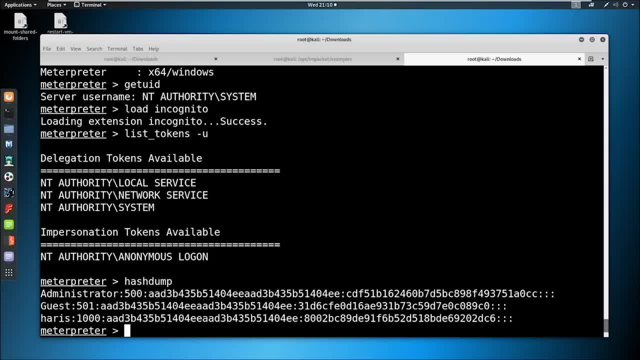 of teaching you to two common internal tactics. Kerberos thing is is obviously one of the more common. that's going to lead you somewhere. But a GPP C password is something you should be checking on pretty much every assessment Because that does lead to easy win You would. 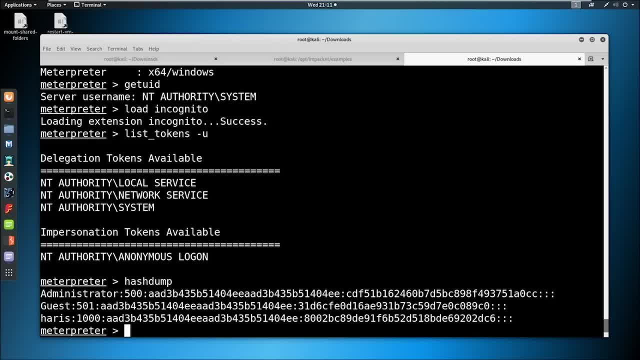 be surprised how many companies have their passwords stored, or even if they've migrated or updated somewhat In an older password that is similar to what their current password is. So any password that you can get is absolutely relevant. So, with that being said, in this stream being all kinds of screwed up, we still 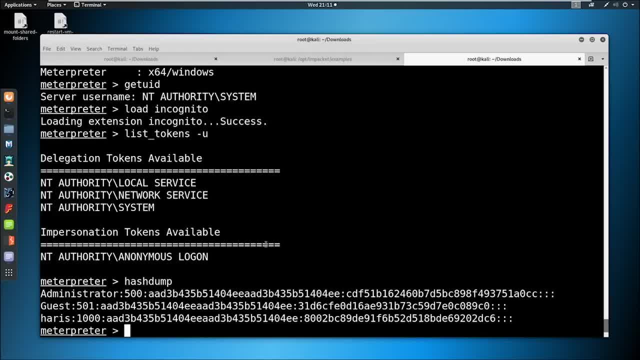 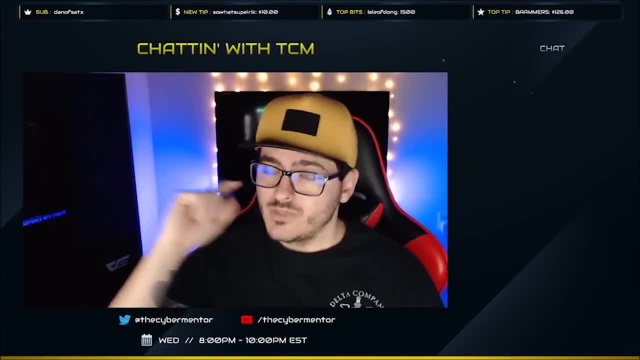 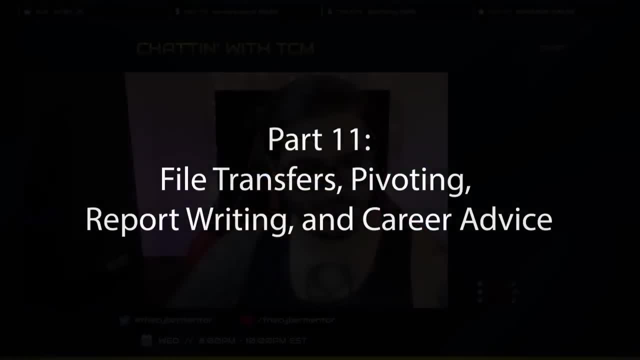 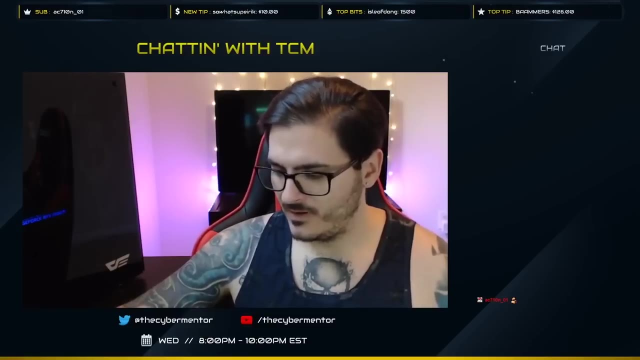 finished 11 minutes past schedule, So that's not terrible. I am going to change my screen over to IRL And we can. we can talk shop for as long as you guys want to. probably hard stop at 10.. Okay, so so far it's pretty good. Let's see what's going on. Let's see if we can see the 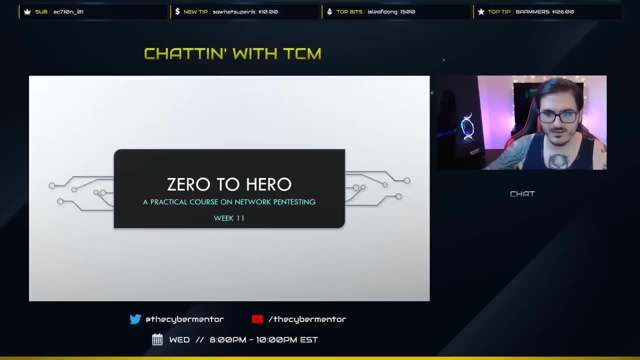 button. Let's go ahead and actually just get started. My dogs are going crazy, So that's awesome. I forget what buttons. there we go, Welcome, Welcome. Unless you want to see my pretty face, we can do. Can do that. There you go, That's not too bad. Welcome to the last episode of zero to hero. 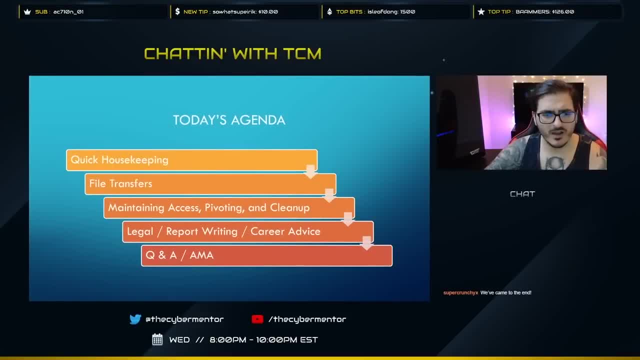 We are week 11.. You've made it to the end, So we're going to do some quick housekeeper. You're going to want to always check out all my videos. We're going to go ahead and do some housekeeping. We're going to talk file transfers. We're going to cover some cool little tricks that. 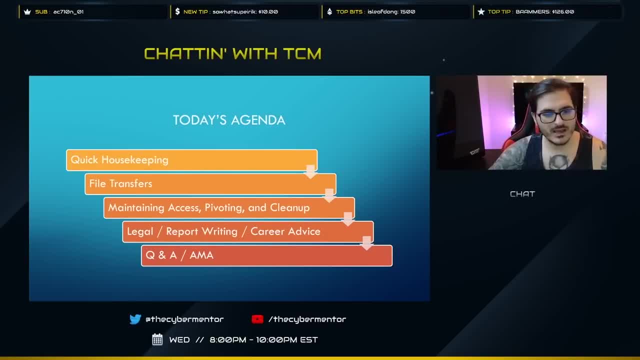 I like file transfer wise, Maintaining access, pivoting and cleanup. We are going to do a lab on pivoting. We're going to talk maintaining access and talk cleanup And I'll get into that and reasonings why Then we're going to cover legal, We're going to cover report writing And 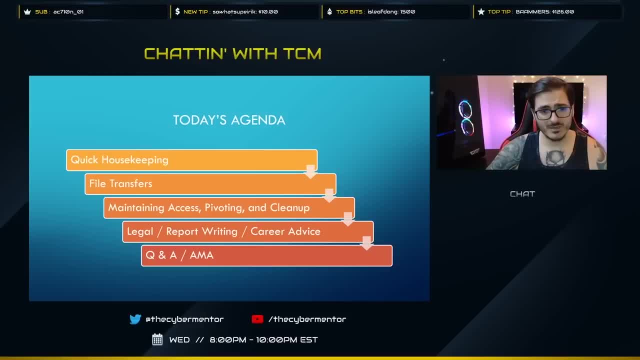 finally, we're going to end on career advice, So we'll talk some legal documentation. I'll cover that example report that I put out- If you haven't seen it, now's the time to talk about it- And then I'll give you my career advice tips, etc. Tip my hat and sign off. So we'll do Q&A. 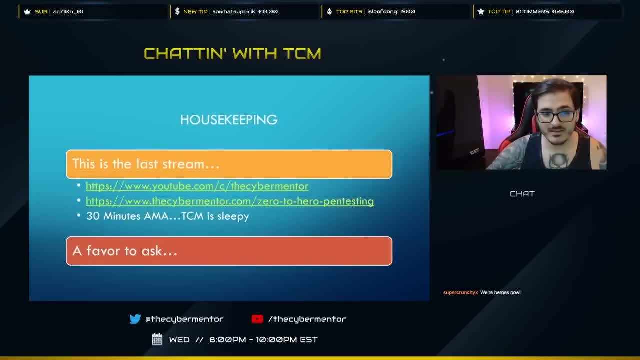 AMA at the end. Let's just go right into the housekeeping. So, like I said, this is the last stream. Immediately after this stream, I will be breaking some protocol and I will be uploading the stream onto YouTube. There's a 24 hour waiting period. I'm just going to YOLO out. 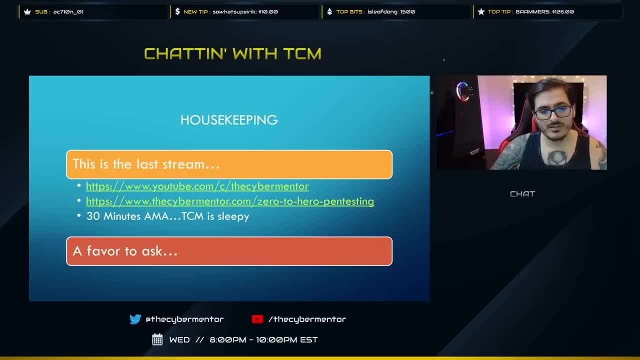 I'm also going to be doing a little bit of a live stream. So I'm going to be doing a little bit of a live stream. I'm also going to be putting it on the zero to hero pen testing on the cyber mentorcom. So if you're looking for that repository, it's on there as well. The course. 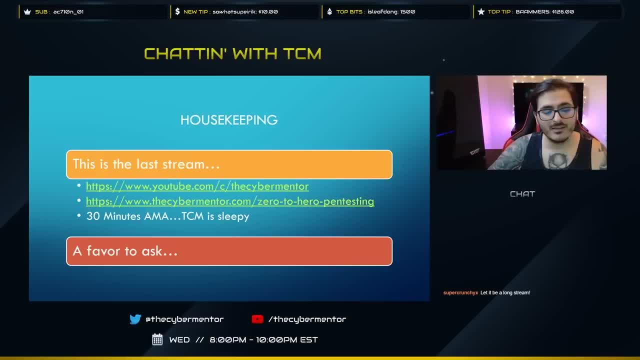 will be full and we'll be done tonight. 30 minute AMA- Two reasons why I am on three and a half hours sleep. I want to party so bad with you guys, but I have a flight at six o'clock in the morning. 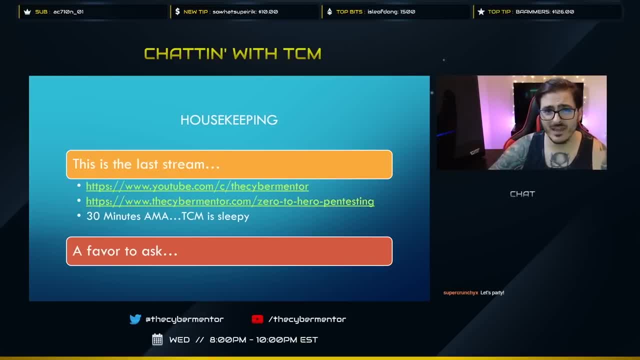 As of just a few minutes ago, I got a text message saying that they may have canceled the flight. So that's great because we've had this book forever. Um, my wife's handling that right now The flight doesn't say that it's canceled online. 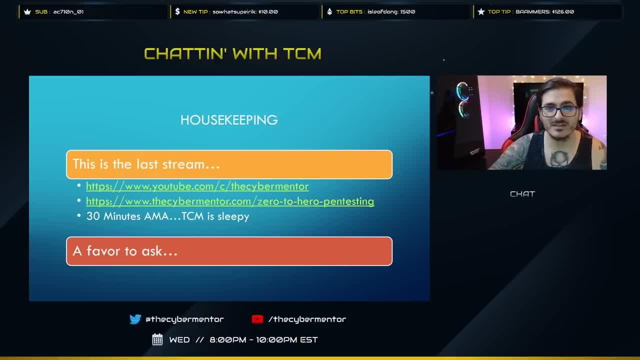 but the text message said it was. So she's on the phone dealing with Southwest airlines right now. Um so, as of right now, potentially leaving at six in the morning. So I'm drinking my monster on three and a half sleep. You guys ask me all the time how do I get all the work done? It's. 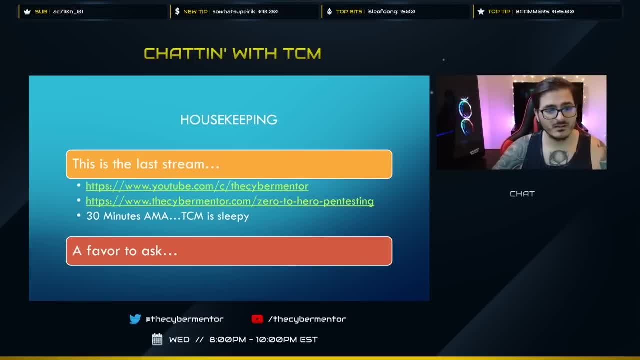 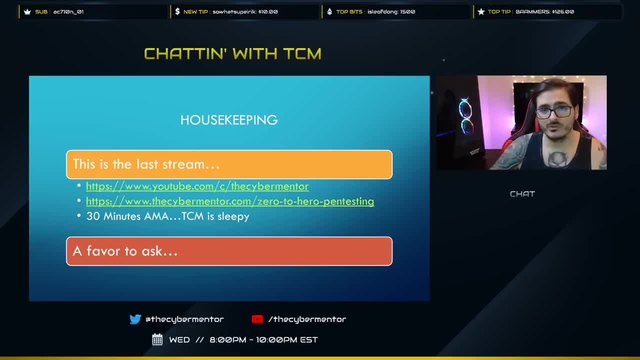 super chill chat. Uh, what we'll do is we'll we'll drink, we'll hack things, We'll we'll have fun. I'll try to pick a different topic that we haven't covered before. Uh, something a little. 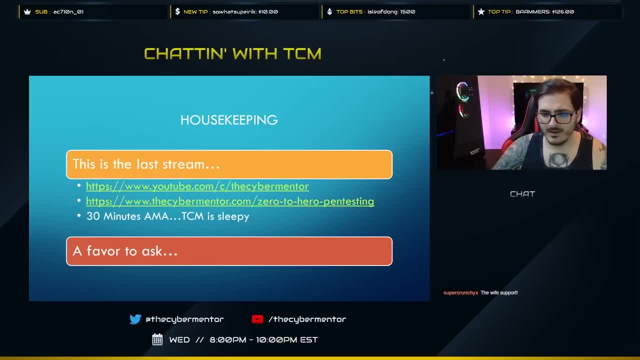 different and we'll just have some fun with it. Uh, so, other than that, a favor to ask of you guys: if you guys are enjoying the course, if you enjoyed your journey, please do consider leaving me some feedback. Um, you could leave it for me on discord, on LinkedIn, on Twitter, I would. 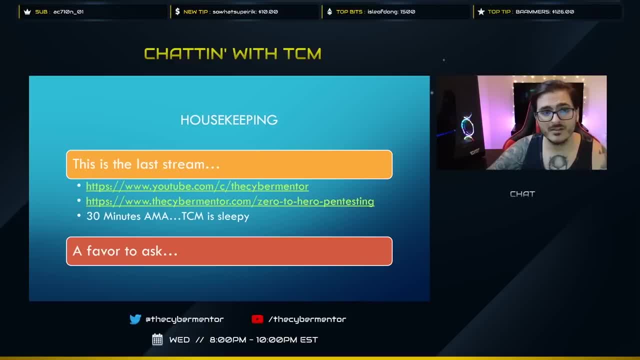 greatly appreciate that Many of you already have, and that's awesome. Um, full disclosure. I am planning and to do this course again, uh, in a paid version, which is just going to include some more updated material. It's going to have an actual lab built out to where we can VPN into it. Um. 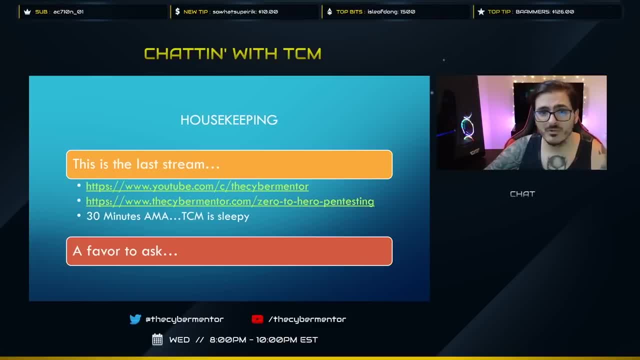 so you guys got the free edition. free edition covers pretty much everything I wanted to cover. The lab is just going to be a little bit more upgraded, Uh, and I would love to use some testimonials if you guys don't mind that. So, um, 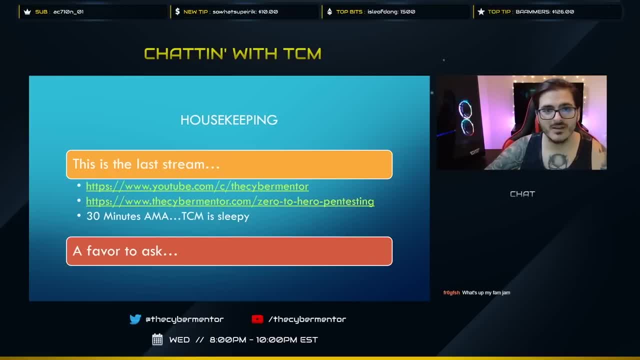 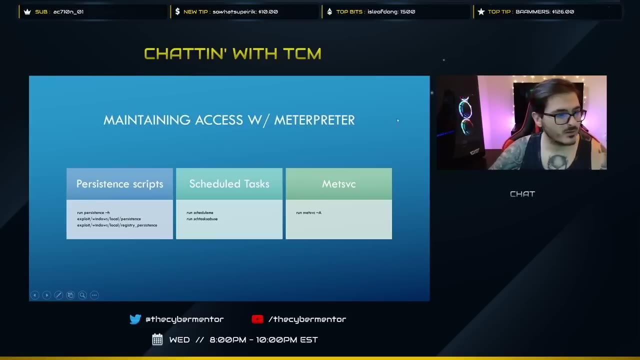 that's my only ask of you guys. Other than that, tell a friend, say, Hey, you know, uh, I, I enjoyed this course. You guys should check it on YouTube or whatever. That would be great, Uh. so other than that, let's go ahead and just dive into our lessons. So I've actually 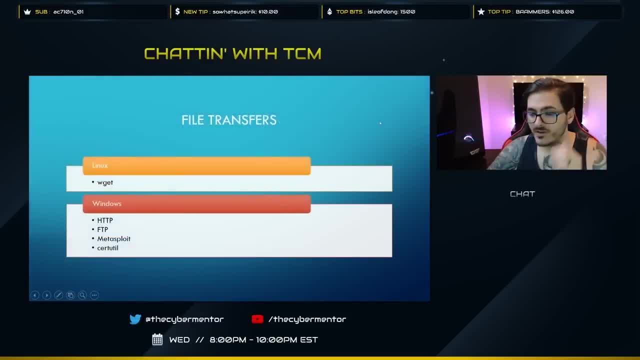 put that in the wrong spot. We're going to talk about transfers first, then we'll talk maintaining access. Um, so if you are looking to take the course, the course will have a discount for students, first responders and military vets. military active doesn't matter. 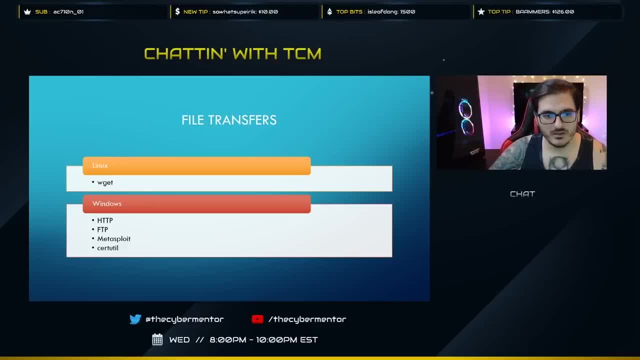 Um, you just gotta let me know ahead of time, and, um, we can work it out. It's gonna be 20% discount, if that's if you guys want to retake this course, Uh, but anyways, so let's go ahead. 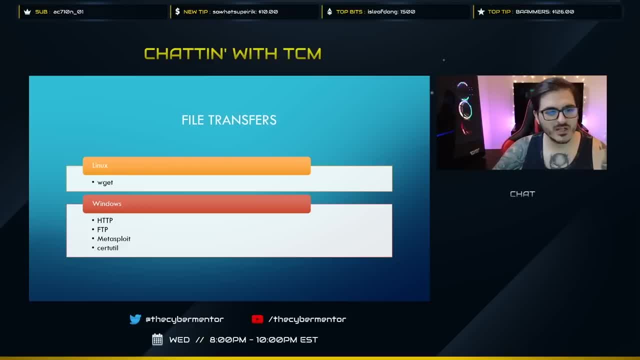 and talk file transfers. So tonight we're going to do file transfers with Linux. Typically, Linux file transfers include uh, w get. So we're going to look at w get. and then we're going to look at some Windows tools. We're going to look at HTTP, FTP, Metasploit, CertUtil- Sick of the mind's already. 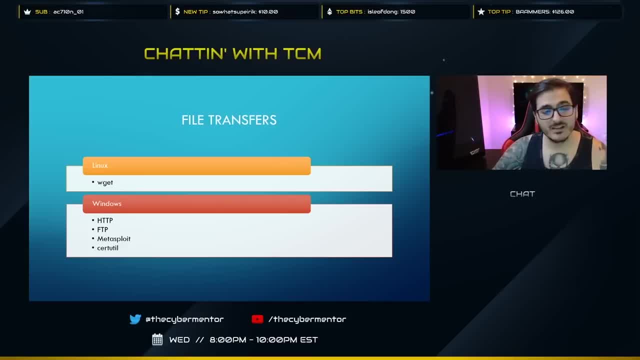 getting ahead of me with um tools. Uh, my disclaimer here is that these are not all inclusive. There are many more, um many more tools that you're going to be able to use, uh, for file transfers. These are just some of my favorite ones. There's PowerShell, there's SFTP, There's 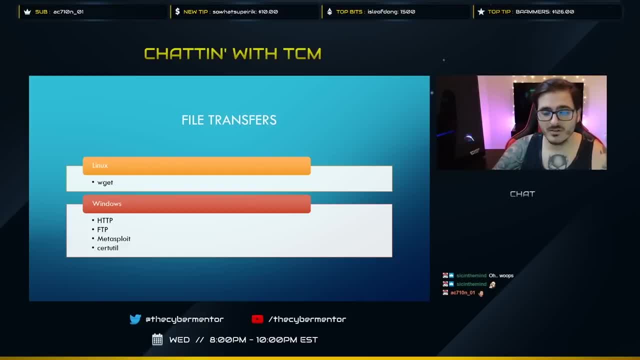 all kinds of cool little tricks that you're going to learn along the way. I'm just going to show you some of the basics, So let's go ahead and get started. All right, so let's go ahead and get started. So, um, and hopefully you learn a couple of cool little tricks, especially with what we're about. 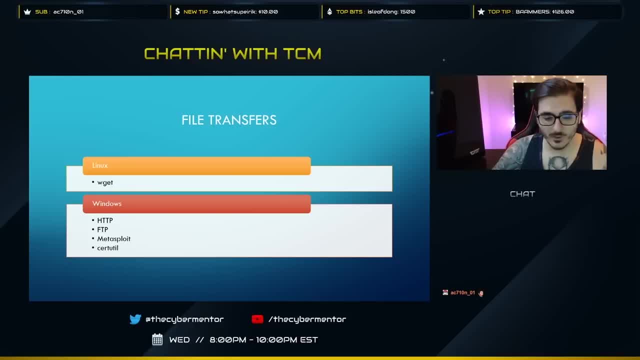 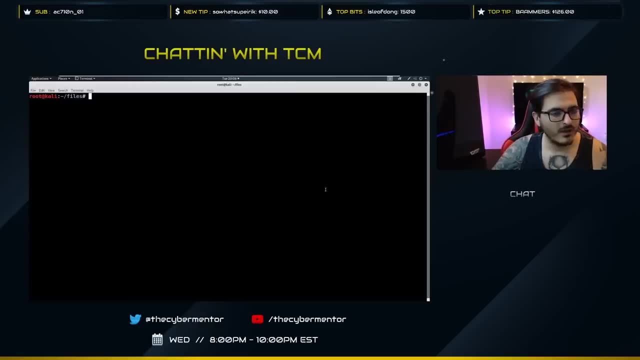 to see in uh in our file transfer lab. So without further ado, I'm going to open up my VM here and we're going to start with Linux. So with Linux file transfers we've already covered. w get right, We can go pull down a file um off the web if we want to um. 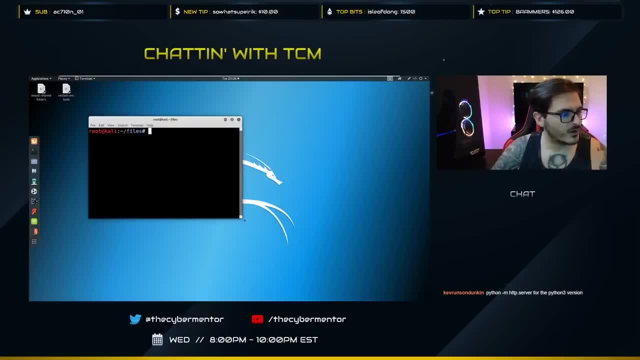 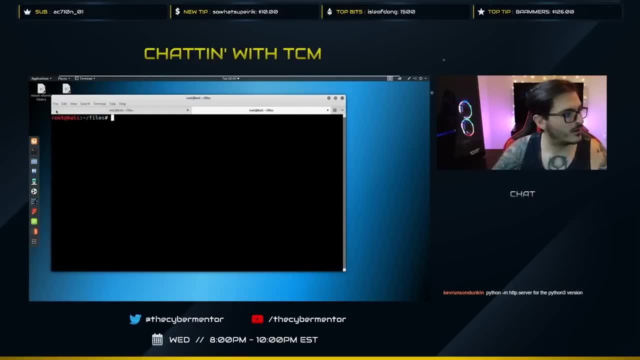 you know, we could actually pull a file, I believe, from ourselves, So we could host up a file. Let's try that, And so all I'm doing right now is I am hosting. um, I've got a folder called files and 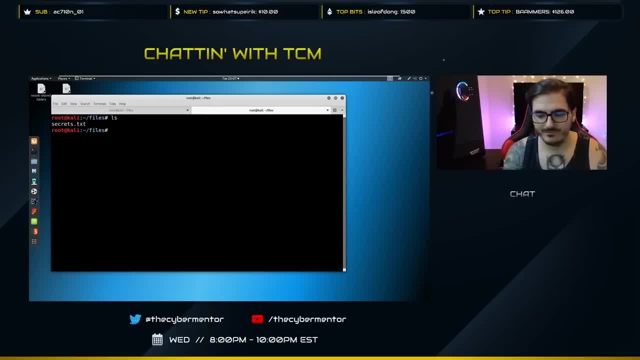 we just say LS. I've got a file called secrets in there. literally nothing in there, but something that says secrets, And what we can do is we could host a Python server now. remember I covered Python servers back during Python lessons, uh, but in case you forgot, 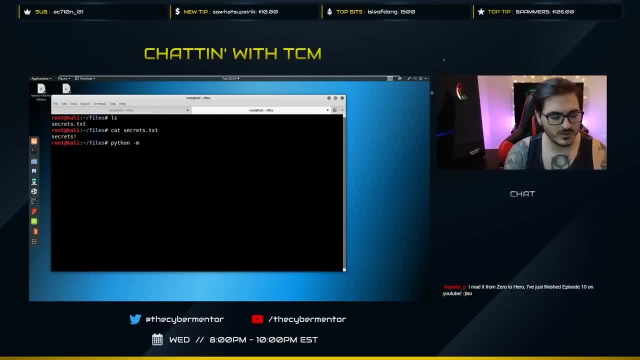 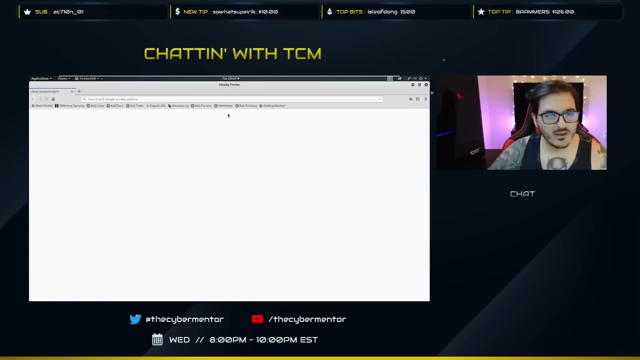 Python dash M here and we are going to do simple HTTP server and you could just type in 80 for port 80, let that run. So anything that's in this location here, the secretstxt is going to be out on the interwebs And so all you would do is go into your interwebs and you can go to your own IP. 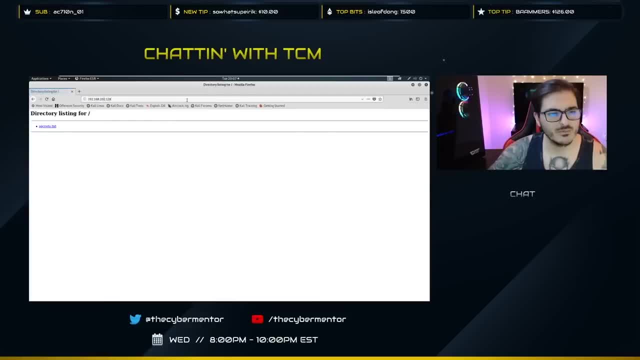 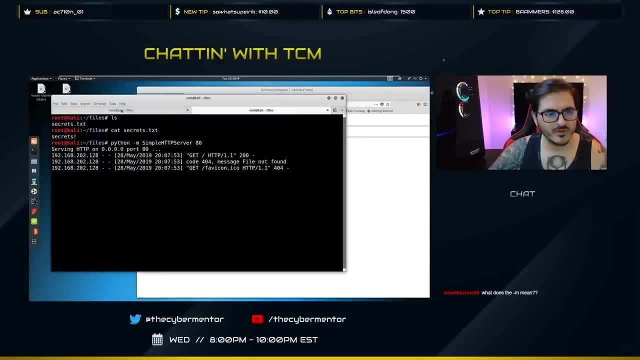 address. I'm sitting at 202.128,, I believe, today. So we got the secretstxt here right And if we come over here, in theory we should be able to W get our own file. We get to say HTTP double slash, slash, 202.128, slash, secretstxt, And you can see that we grab. 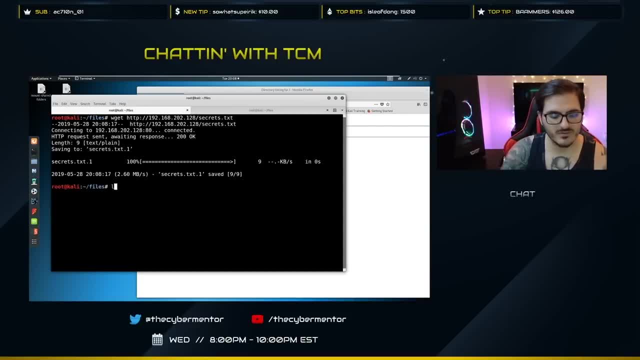 secretstxt, and I put it as a dot one because it already exists in the folder, And then if you come over to here, you see that it actually shows that we grabbed it. So somebody came in here and made some sort of grab, So we 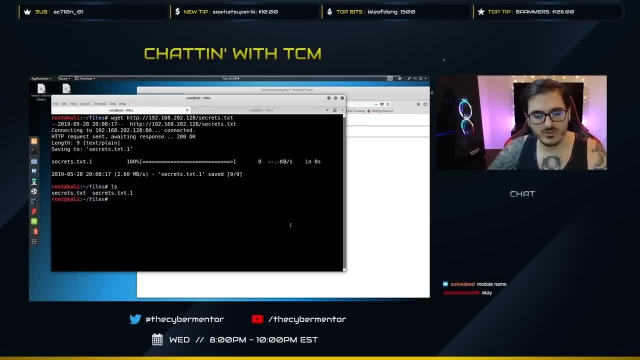 know that W get works. Now there are some additional cool tricks that we can do, uh, with W get, And one thing that people don't know is that you can actually push out files from W get. Okay, So let's cancel this HTTP. 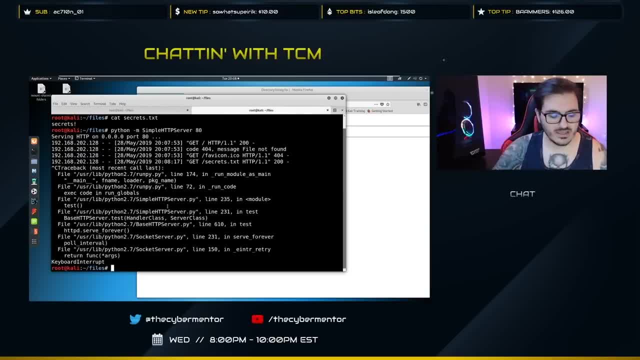 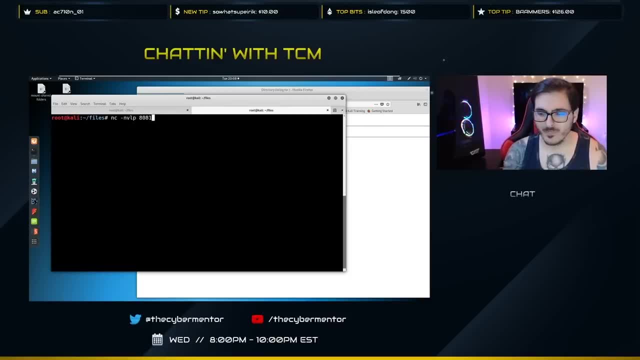 Server here And let's do instead. let's set up a net cat listener. So we're just going to say net cat and BLP and let's just put it on port 80, 81.. Okay, So now imagine this scenario: You are on. 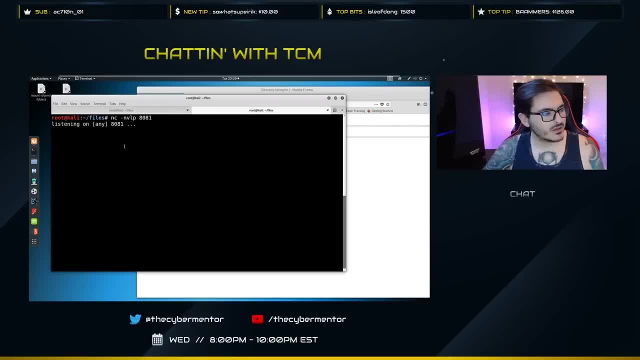 a machine that you have exploited. You set up a listener here And what you can do with W get is: there's actually this module in there. If you say dash, dash, post file, like that, and then let's just say: we want to get rid of this. secrets, right, Secrets dot text, And we want to 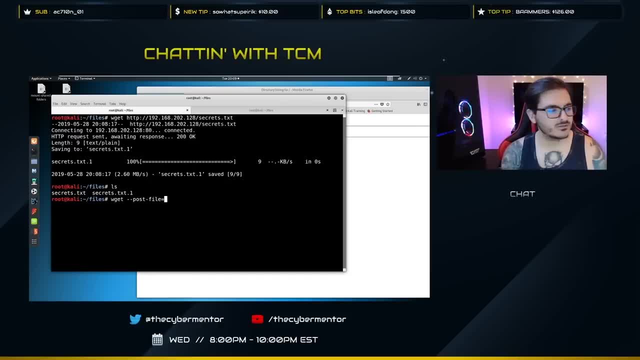 we want to send it out. Actually, let's do something better. This is more practical. Let's say, we want to send out the Etsy password or the Etsy shadow file, right, You can do this, and then you just type in an IP address. 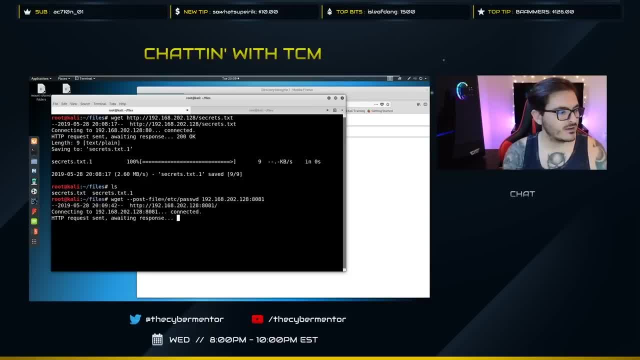 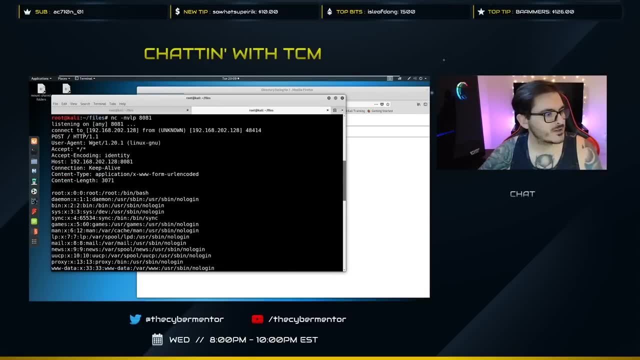 one, two, eight, and then you type in the port number. at the end of it says awaiting response. But if you come over here, look what just came through. So it comes through like it is a uh with the web header right, And then I've got the whole. 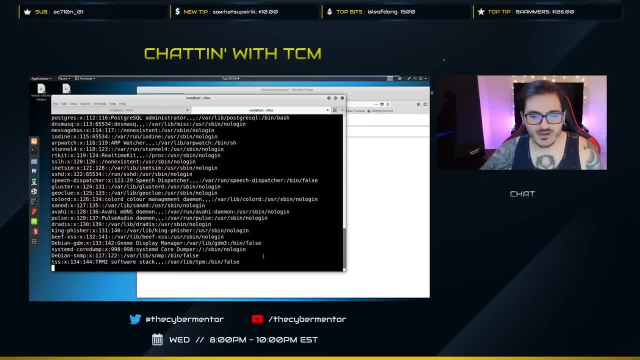 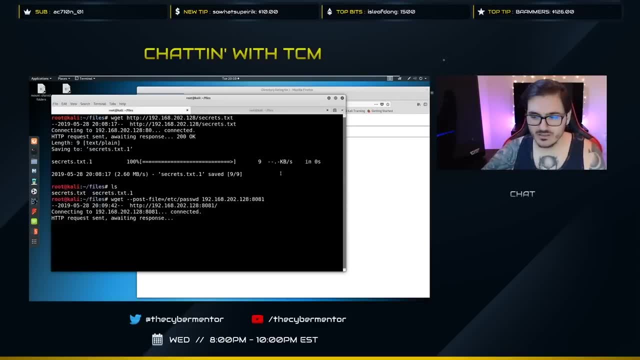 file that just came through here. So this is a quick way to dump files off to yourself that I feel like a lot of people don't know about. It's pretty neat, Um, so that's a neat little way to transfer files back and forth using W get with Linux. 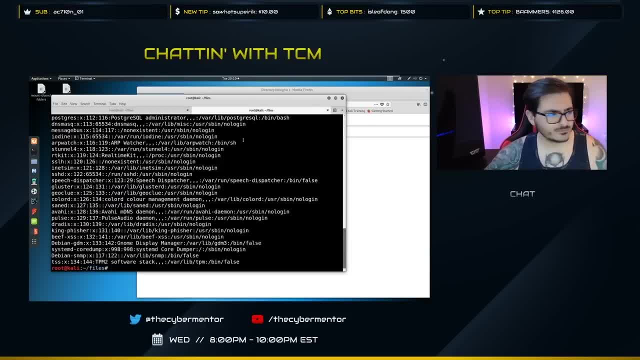 So let's talk about windows while we are at it. So you just saw, um, I talked about HTP. You just saw me spin up a file. I'm going to show you how to do that. I'm going to show you how to do that. 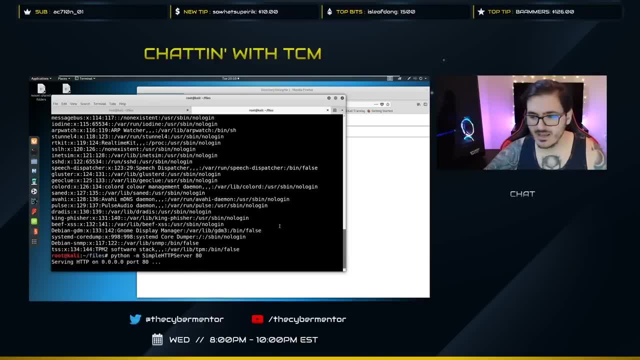 So we've got a file server here, So Python, dash M, the M. somebody asked for the MS, for it's for module, So we've got the dash M and we're just listening on port 80 for any traffic. Now, if we were on a 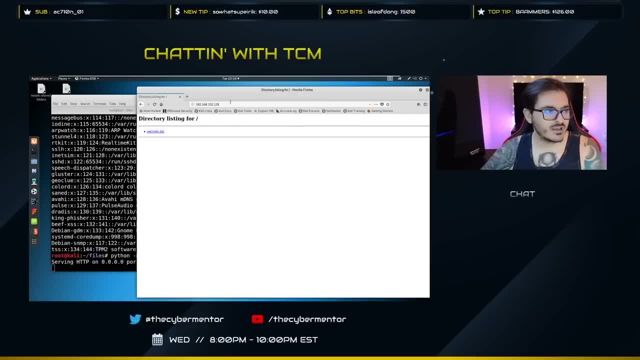 RDP machine, then we would just come in, right. We'd say, oh, I'll just go down to the web server, That's easy. Um, we've got GUI access, right, And then we'll just download the file. And if we click, 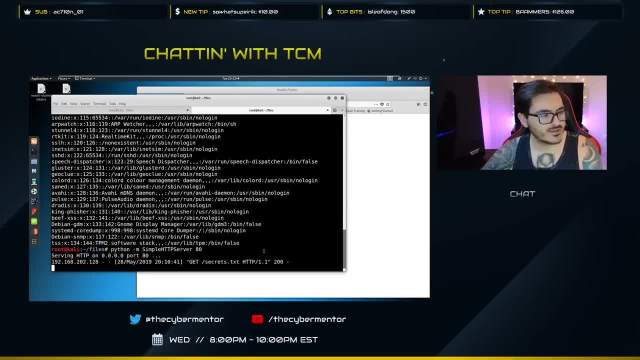 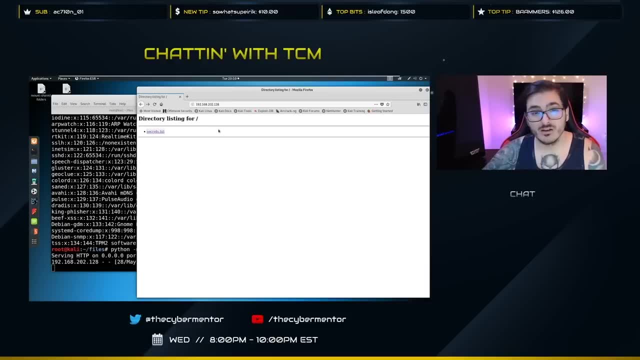 on it, you'll see that traffic comes through and somebody made a get request to that secret side Text And it just says secrets. So that's a common way, a really common way If you've got access, uh, GUI access to a machine. 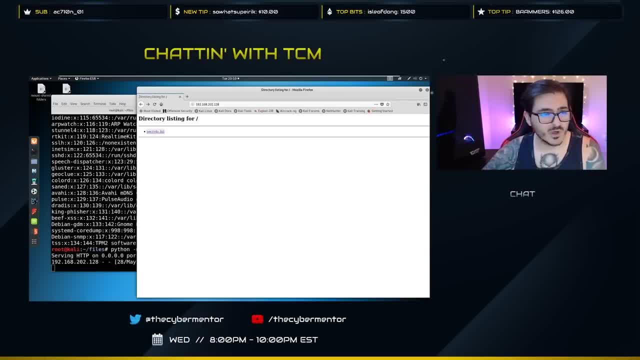 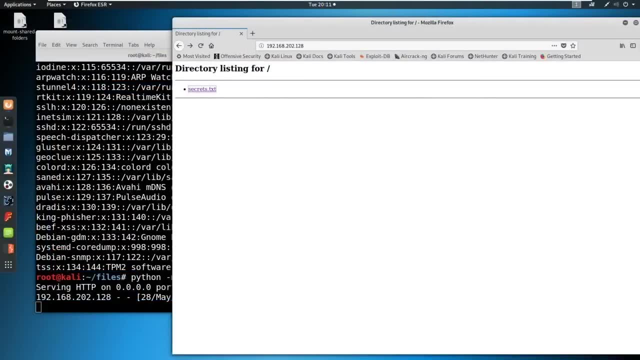 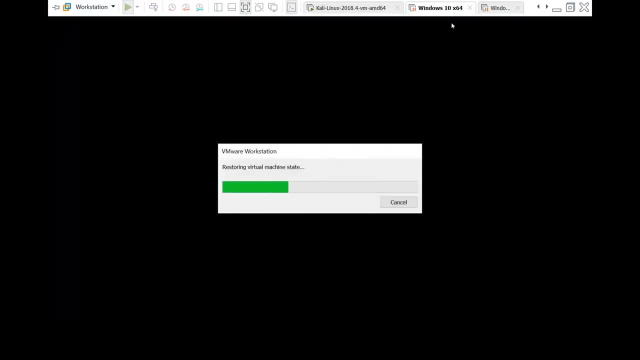 uh, but the rest of the ways I'm going to show you are for if you don't have GUI access to a machine. and let me actually make, uh, this full screen here so you guys can see. So I'm going to power on my windows 10 machines, Um, and I've got this lab set up for pivoting, So let me see which. 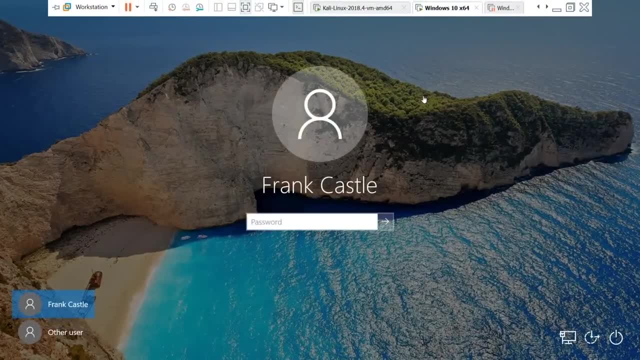 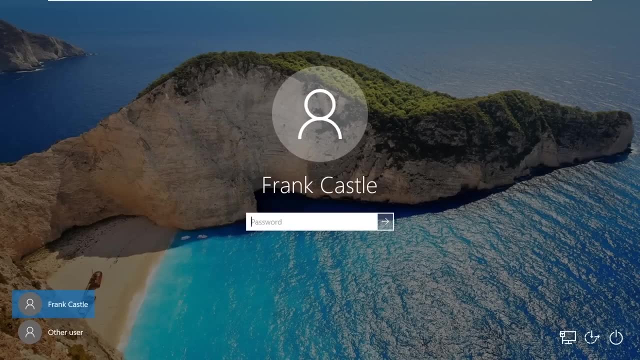 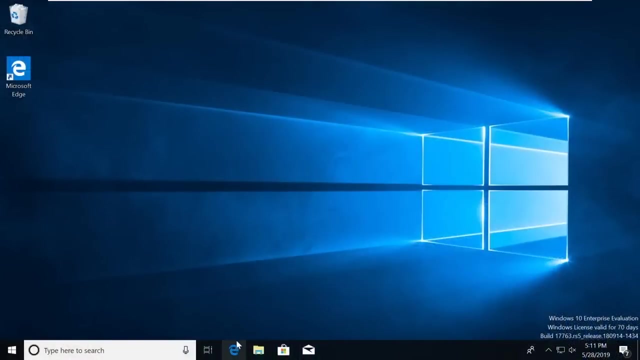 one is which. Okay. So for for you guys, you can log in either one, um, but I'm going to be logging into Frank Castles machine. So this was the first machine that we set up And again from Frank Castles machine, anybody on the network can go to that location. 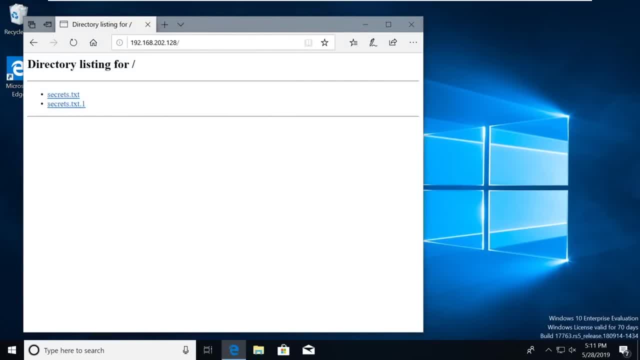 see, I've already got it up, but see, because that text, see, cause that text, that one's in here? Um another thing that we can do while we've got this running. So, um, imagine this scenario: You. 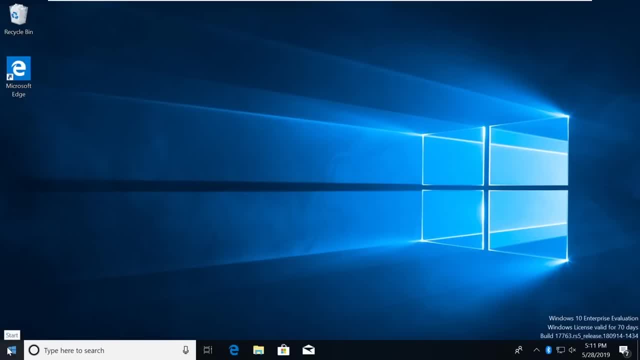 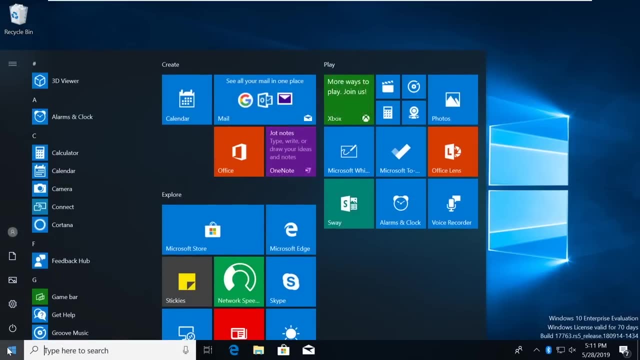 but you do have access via a shell. There is a wonderful tool. Now I will note that this tool has been getting blocked lately by Windows Defender And I've actually gone in and turned Windows Defender off in in group policy. So if you want to do that as well on your machines, 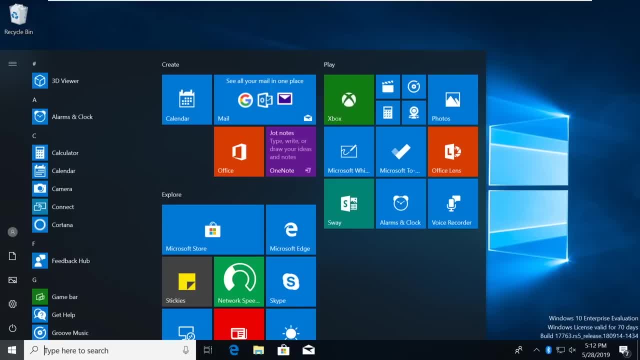 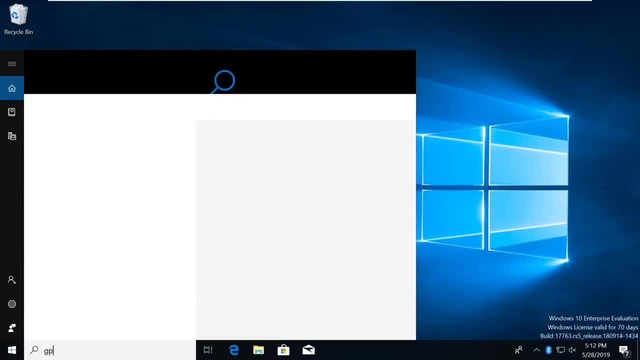 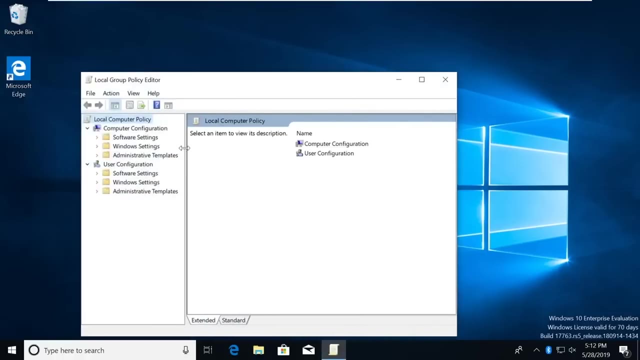 like some people were saying that the machines were, were were turning Windows Defender back on after a reboot, And that is pretty accurate. You can go into your GP edit on your local machine and just go into here And then there's actually a setting if we go into. let me cheat and look at: 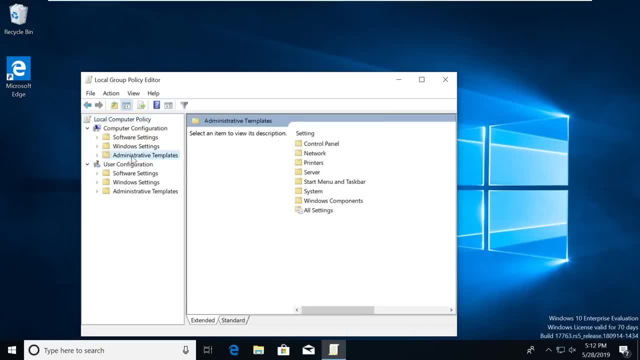 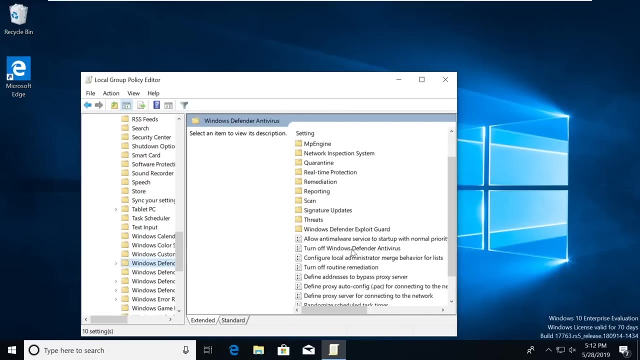 my notes. So if we go into the administrative templates, and then I believe it's Windows components, And then there should be a Windows Defender antivirus right here. So there's this little policy that says turn off Windows Defender antivirus If you double click on that and you say enabled. 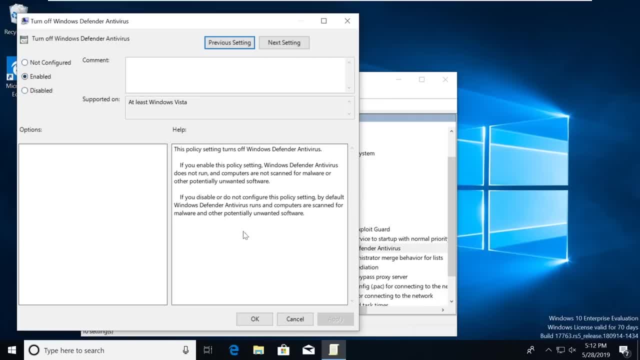 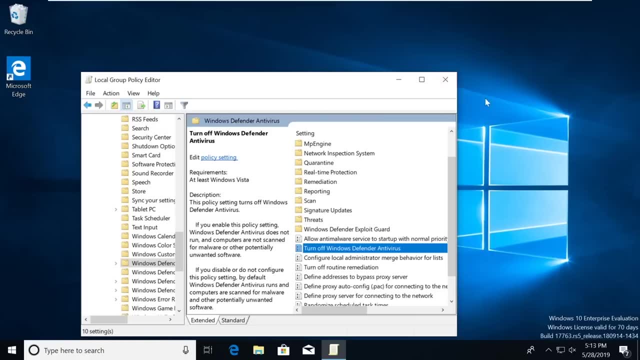 it should be not configured by default. If you say enabled, this will turn off the policy or this policy will turn it off, You just hit OK, then you reboot and you are good to go. So if you want to do that for all your machines, you're more than welcome. If not, you may have to. 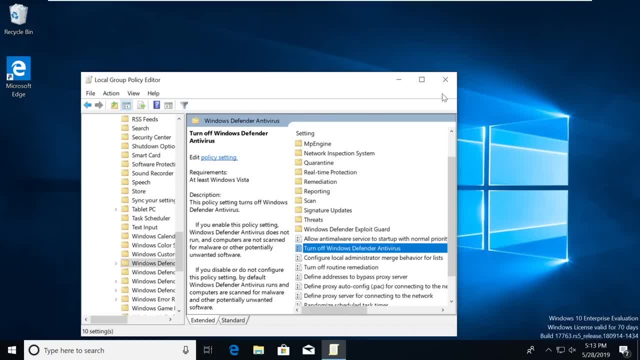 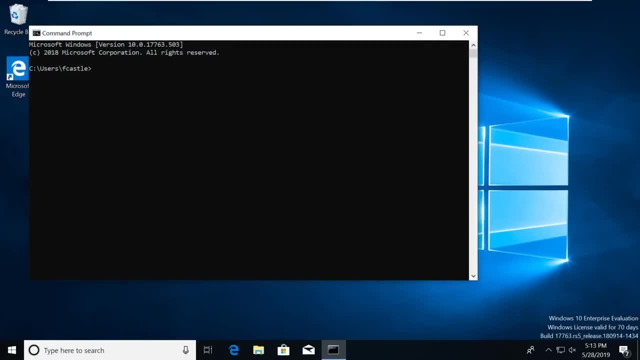 turn off Windows Defender again tonight for some of the activities that we're going to be doing Anyway. so there is a tool that I like to use. If you go into command prompt, this simulates what a shell would be like. What we're going to do is we are going to use a tool. 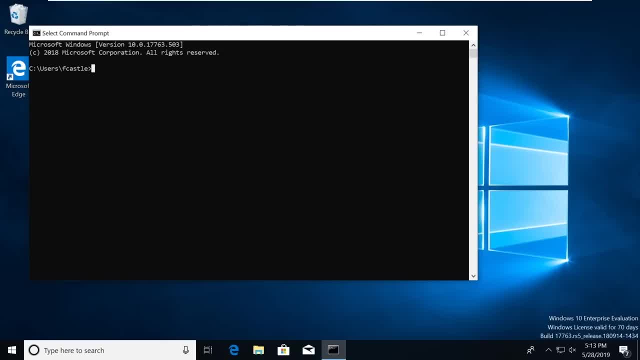 called certutil. This is fairly common and I don't feel like a lot of people know about it. So if we say, apparently I'm not typing in here, we say certutil and it's built in to almost all of Windows. like for a long time now I couldn't tell you where. 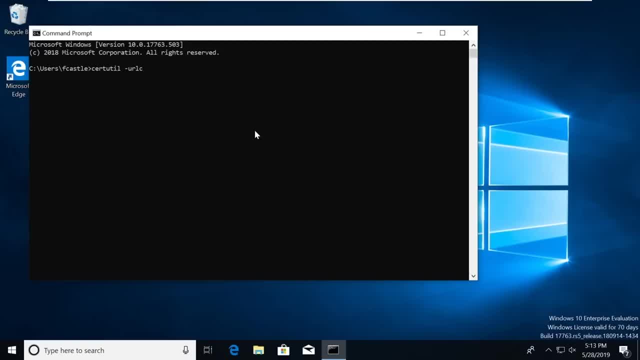 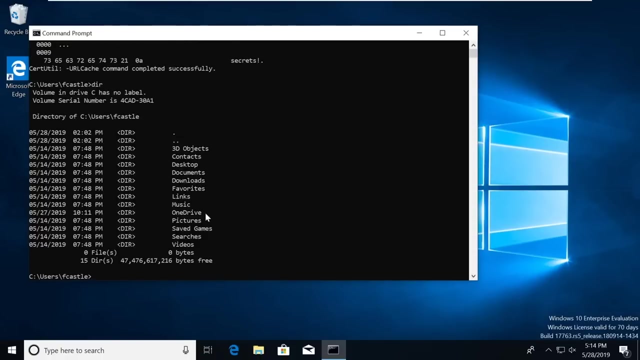 But this is kind of the equivalent of a wget. So you say: dash URL, cache a dash F for file, and then you just grab the file you want. So 68202128, slash secretstxt, pull it down. you say dir and oh, I messed up, You got to name your file, So we'll just call it secretstxt, like this. 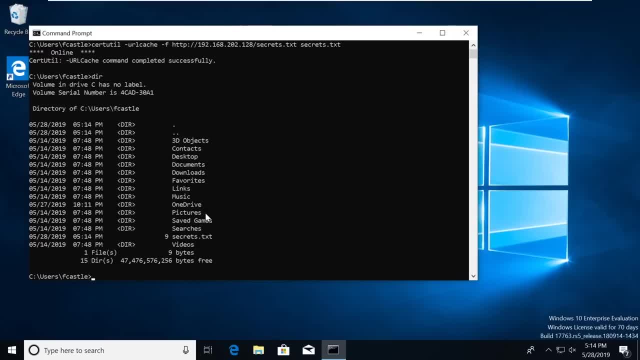 And then it says complete successfully Let's dir. And then you see, the secretstxt is here. we could type it. make sure it actually came over correctly. And he see, it says secrets. So that's a neat little way. There's some more advanced methodology behind this too. 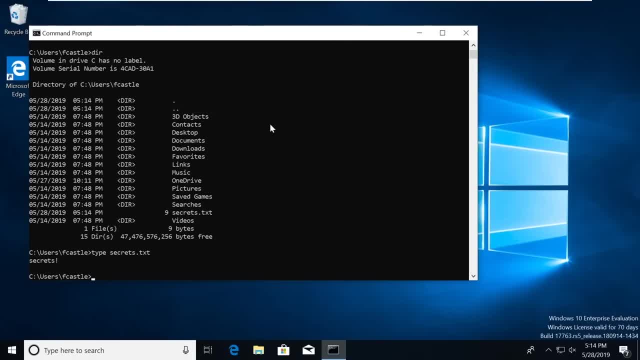 There's actually a way to split the files and then rejoin the files to kind of bypass some antivirus. I've never actually had it work, but I've read blogs on it where it shows it working. So there's some little tricks, tricks on that on the more advanced side. but just know that cert util, especially if you're doing. 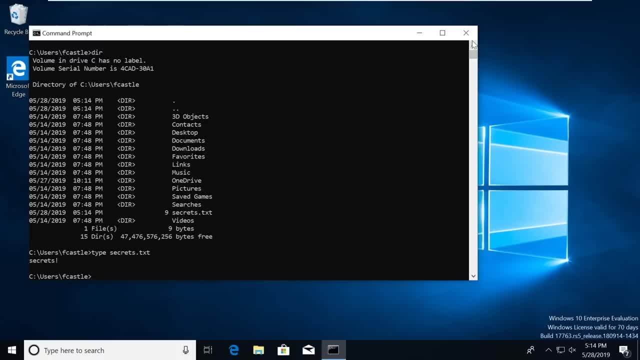 things like capture the flag or, you know, hack the box, even oscp stuff. this is a neat little trick that you can use to bring files over. so on top of that, there is one more trick that i would like to show you, and that is ftp. and let me make sure that is the only trick i want to show you. 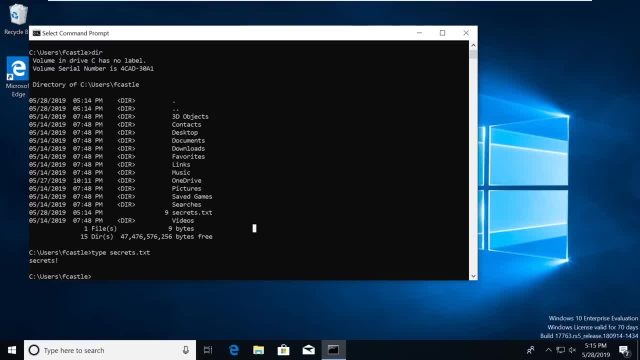 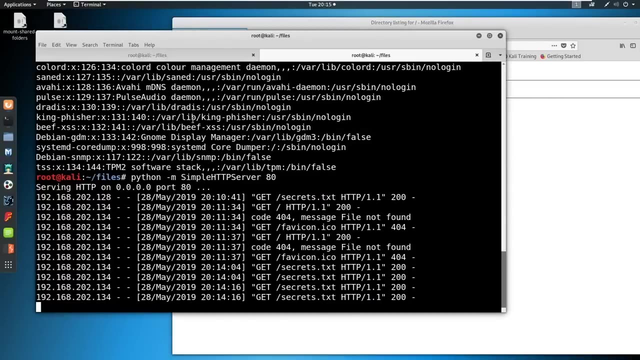 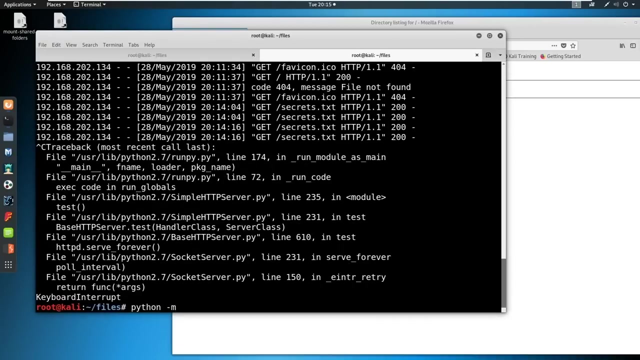 i don't have all my notes up. let's see, uh, where's my powerpoint. http ftp, oh yeah, and metasploit, of course. metasploit, um, so we can also spin up a ftp server. now, if we come back into here and we kill this now with python, we can spin up a quick ftp server module as well. it's called pi ftp, you just. 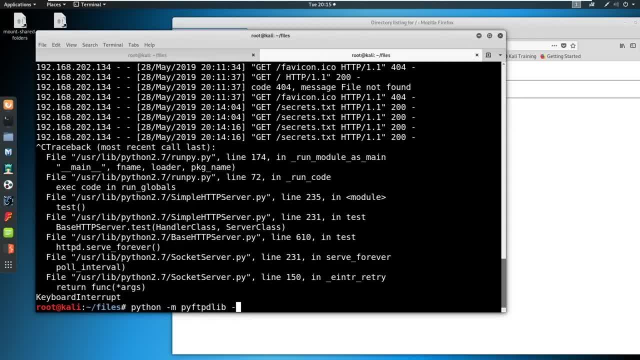 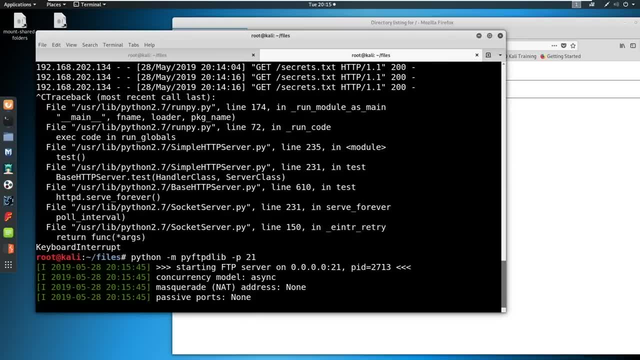 type that out and hit tab and then you do a dash p for port and 21 like this. you start running it. now some of you might be trying to run this and it's not working. um, the reason that would be is because you didn't install it. if you've, 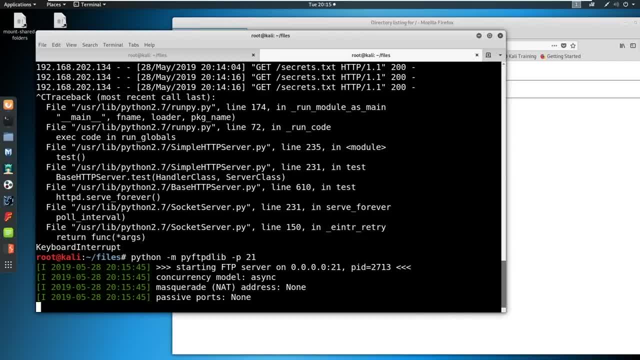 been following from week one. i had you install this either week one or two, one of the early weeks. um, i believe you can just do a pip install of pi ftpd lib and that should get you where you need to be. um, but either way, just like the port 80 web server, we just spun it and it's working. 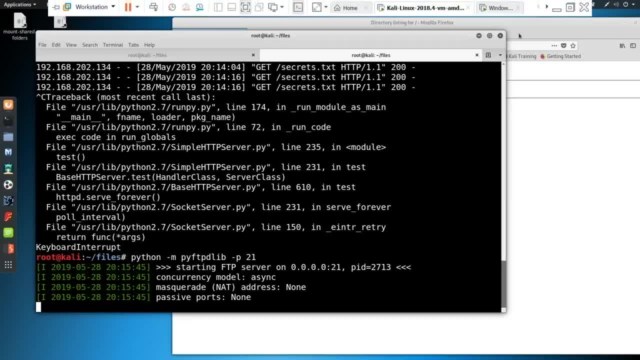 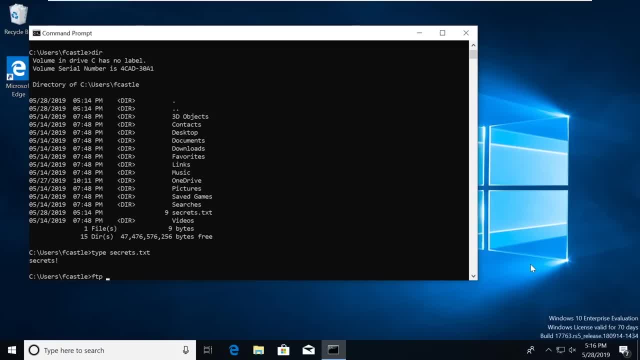 up. this is the port 21 ftp server that we're spinning up. we can come onto our windows shell and we can say ftp and then type in the address you want to go to. it's going to say: okay, you've connected. what's your password? username, password- just type in. 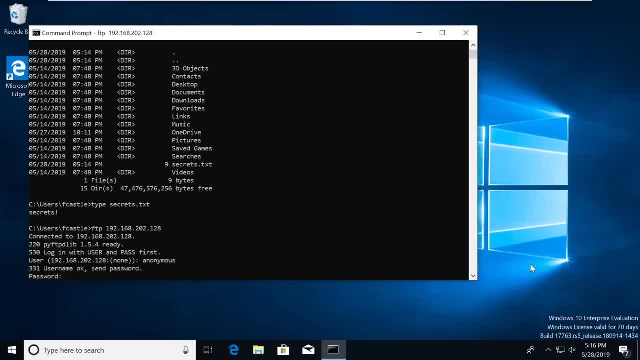 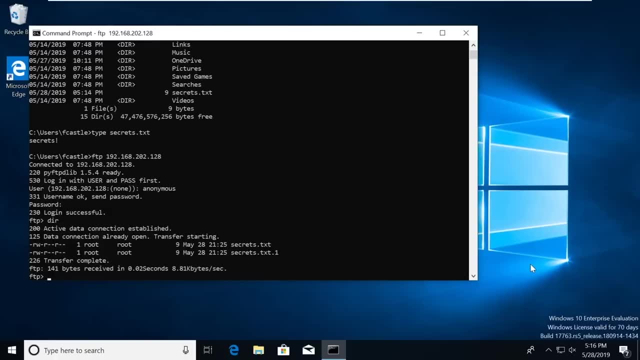 anonymous. anonymous, preferably wearing your guy fox mask right. and then you are here so you could say: der and again, same thing. um, it's going to put it what all the files that's going to share are right in the folder that you spin it up in. so again, we have the secretstxt you could type in. i think it's. 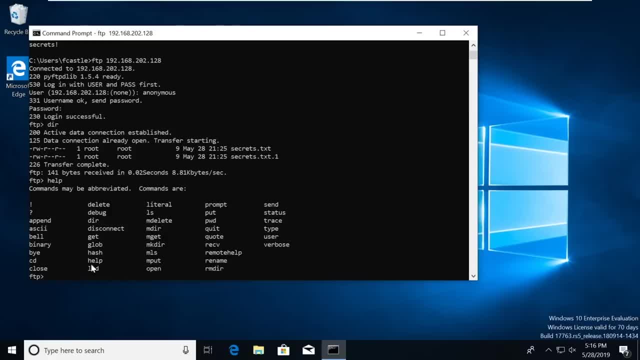 help to find all the things that you can do. but you can put files in here with put, so you can transfer files out, and you can also get the files from this folder as well, so you would just say: get secretstxt. so it's fairly straightforward one of the easier ways to transfer files. 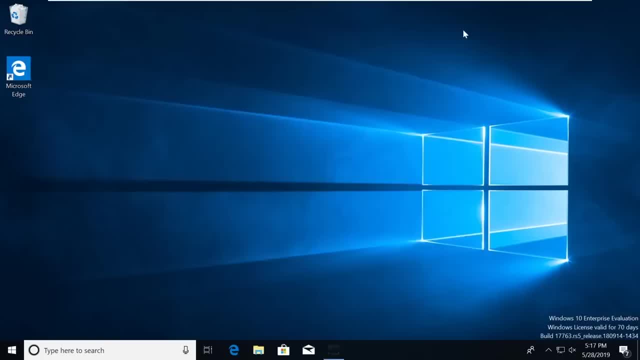 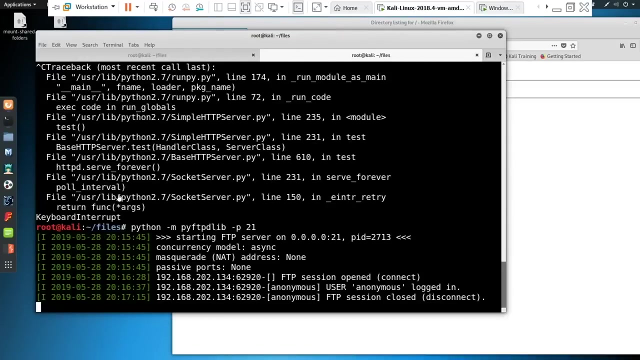 out, and you can also get the files from this folder as well. so you would just say: get secretstxt, okay. so let's go ahead and exploit, um, our machine again. we've got this windows 10 machine here, remember, we have a ps exec exploit for it. so i'm going to exploit the machine and we're going to 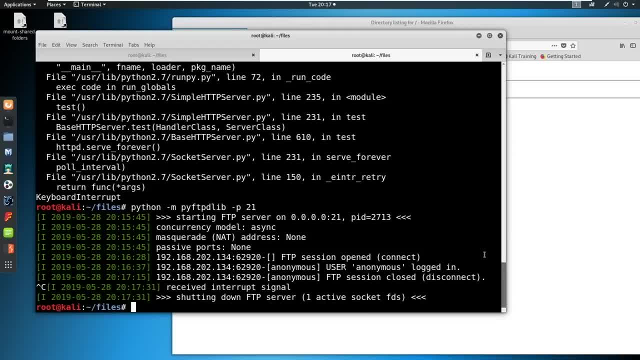 just kill this, and i've got some questions coming through. is there any reason why you shouldn't do it in bash service, vas, tpd start, because that turns it on permanently. this is just an easy on right, so you've got your service up and then you got your service off. it's the same thing with the. 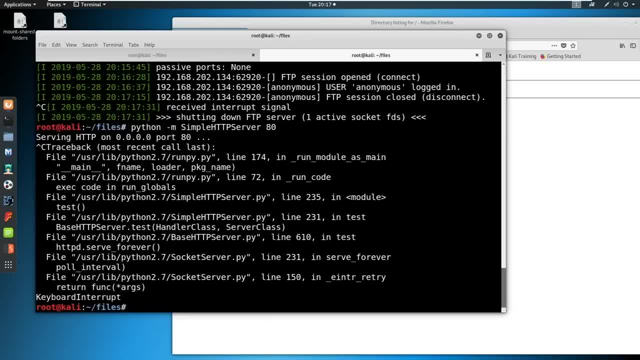 web server, like the web server is running, and then that's not running right. um, the other way is you start up your your web server with, like, say, apache, then you have to go put it in your folder, like you have to go put it in your www folder to share it out. um, here you can just share. 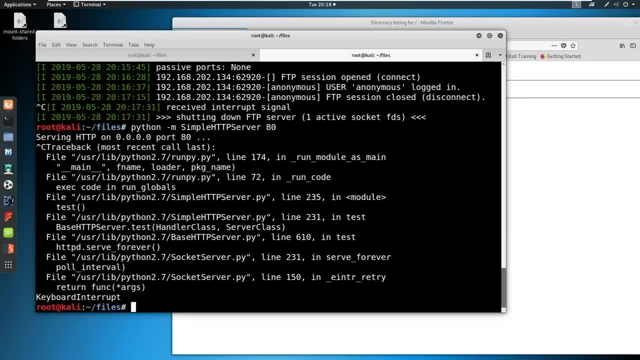 the folder what you've got right away. you don't have to go put things and items and locations you want. it's just an easy spin up, so it's it's instant, and that's this is why i'm going to show you how to do it and that's why a lot of people have moved to python for for spinning up these quick servers. 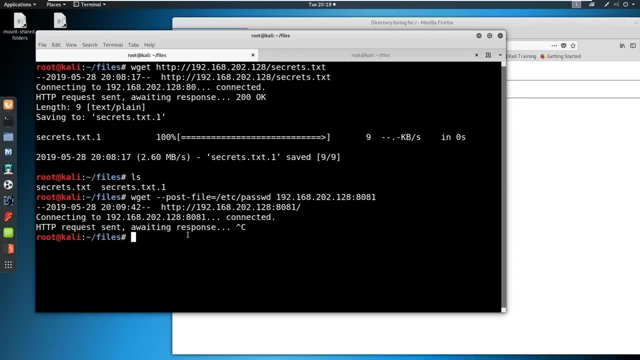 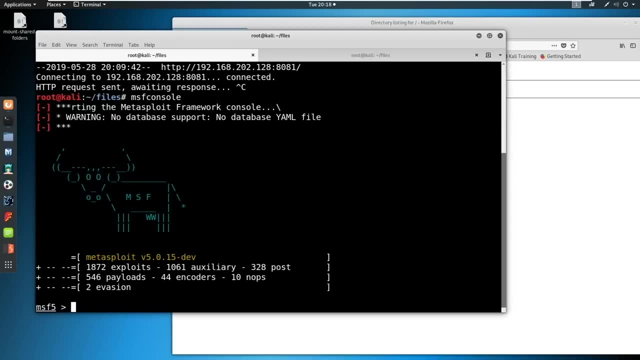 okay, so let's get into. let's get into metasploit. if i'm going too fast, guys, let me know. um, i'm just trying to get through everything tonight and i saw some people came in: hey, jeff, how's it going? hey, dan, nice to see you, man. 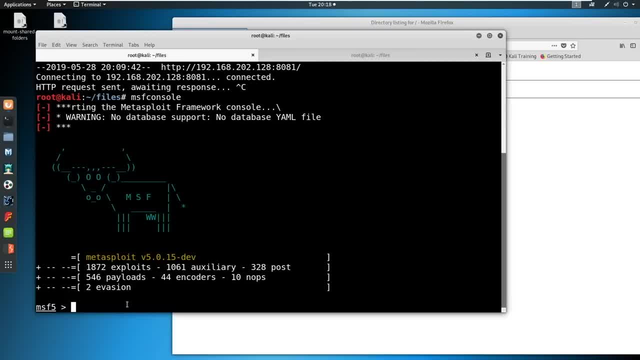 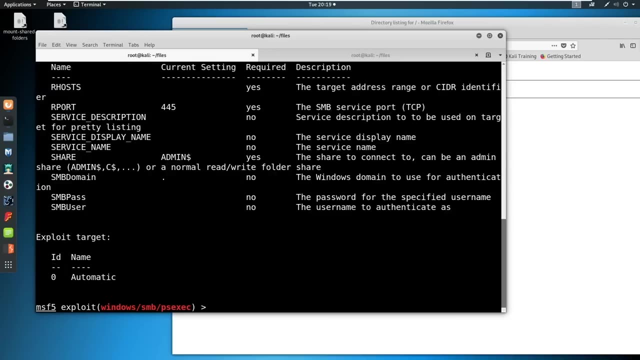 okay. so we are going to exploit our frank castle machine one more time. so we're going to say use, exploit windows smb, ps exec should be familiar from all the previous lessons. we say options. okay, we're going to set our r host. my r host for this machine, i think, is 134. 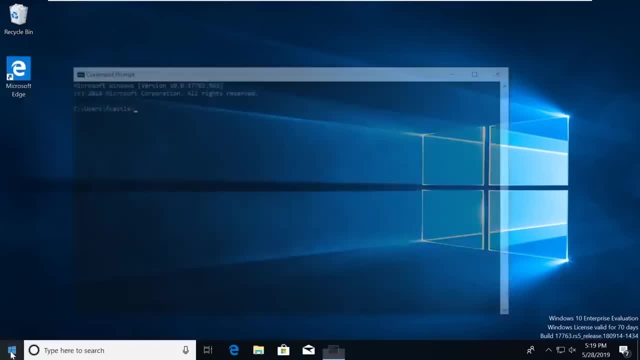 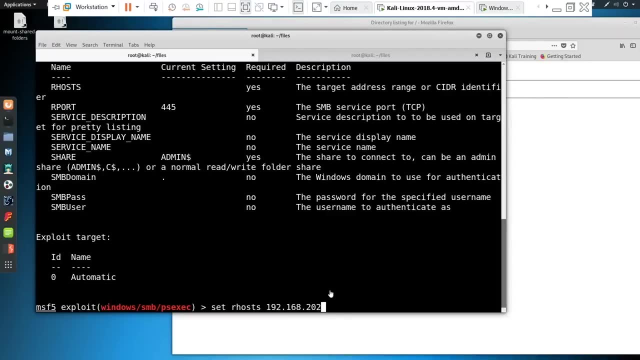 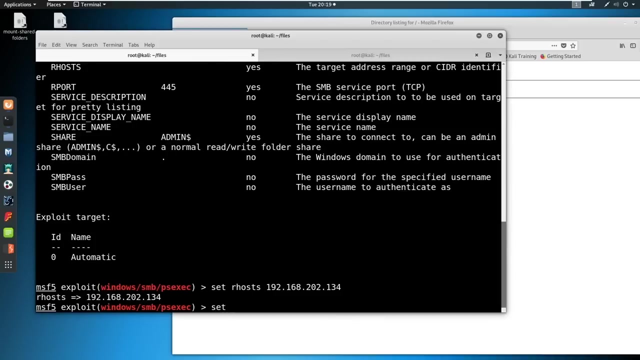 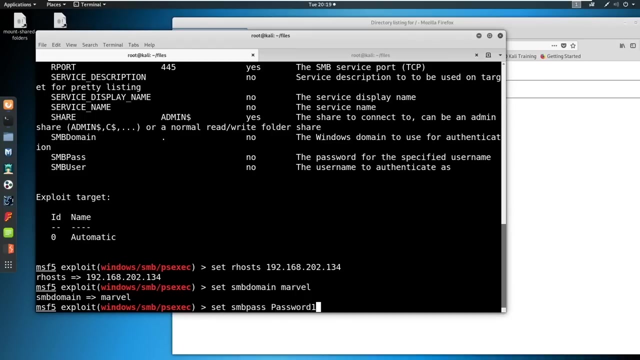 i don't want to be wrong here. okay, we're going to set the m Mongol, it's 202.134. we're going to set the smb domain as marvel, set smbpass as password one, set smb user as f castle and let's set the target as two. 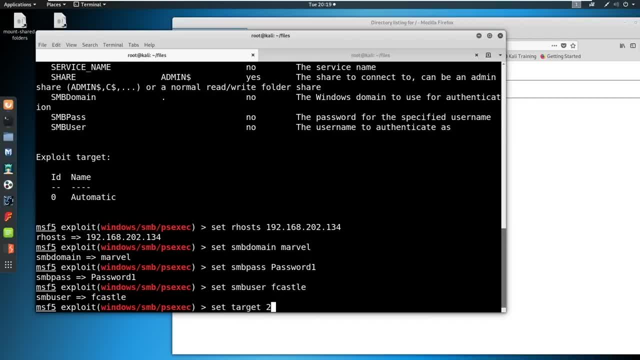 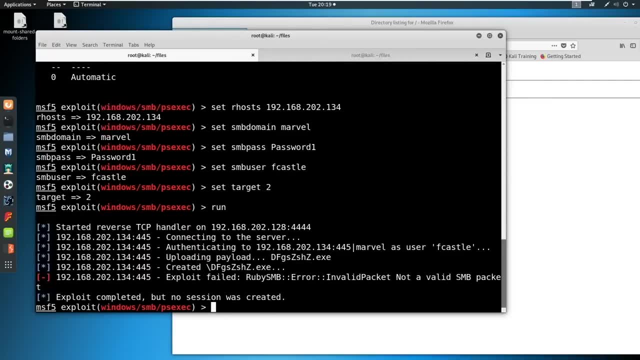 remember it's got the automation, so that's something that you won't normally expect to see anyway. so let's create our new those clashARP, and let's set this down together: name and Inform già, automatic target, and sometimes it works. sometimes it doesn't see if this even works, denied that's. 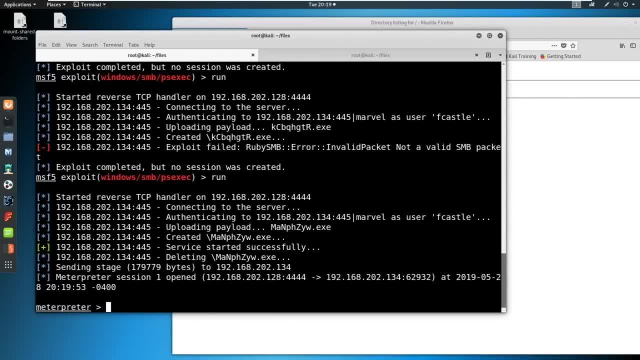 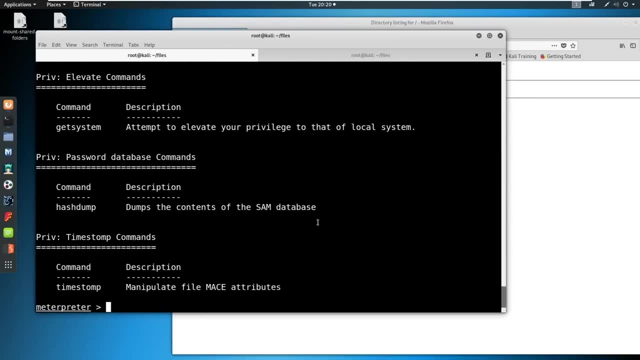 okay, we'll try again, try again, try again. okay, we've got our shell. so one of the nice little features about Metasploit is it's got a lot of stuff it can do. we've been doing pretty much all of our work in Metasploit. it is so robust and so awesome. I'm the biggest fan. skitty, whatever you. 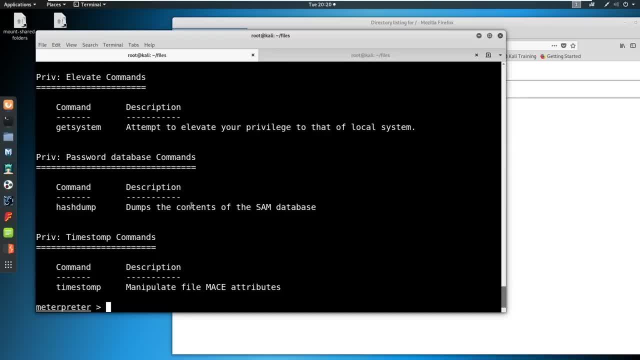 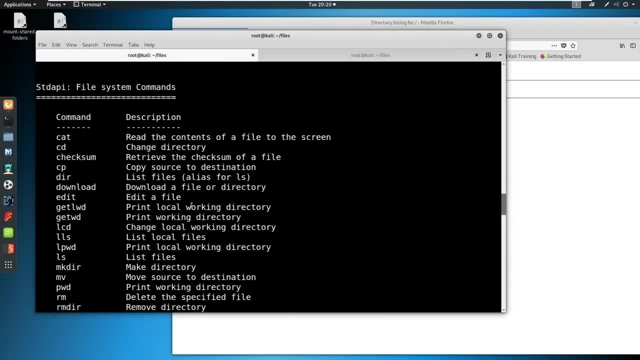 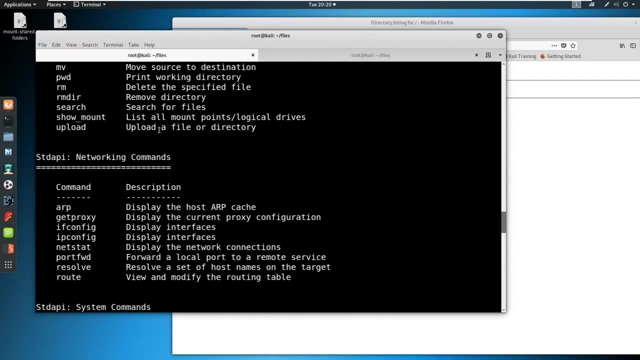 want to call me. when it comes to Metasploit, I'm I'm all about it. so if you come in here and you say there is an upload and a download, I might go buy it. I don't know, I'm not good at seeing things, just just trust me. okay, there it is: upload and download. 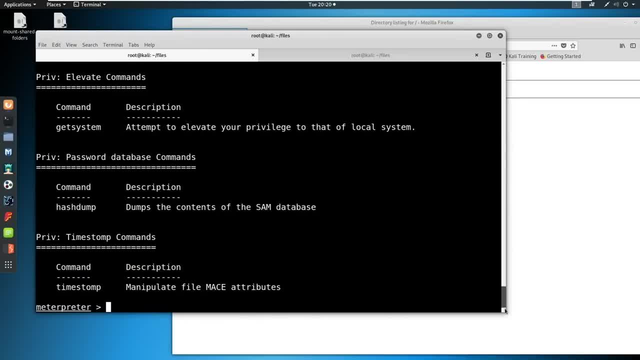 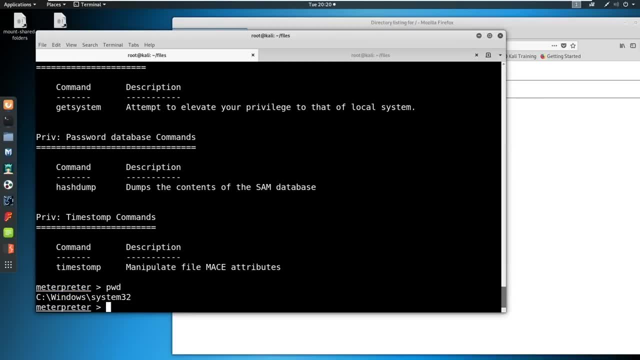 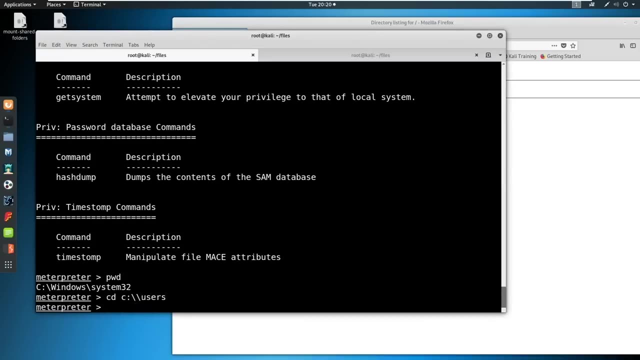 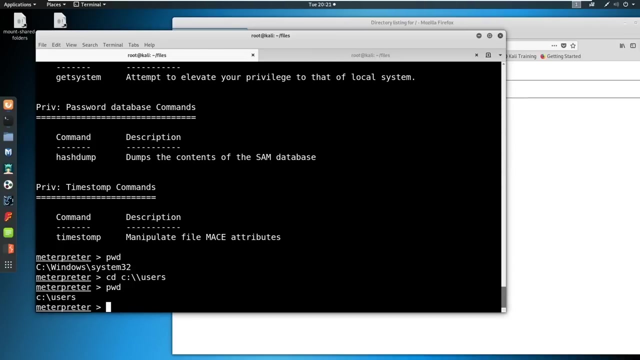 you pretty much have full control anyway here. so you could say like I think it's like present working directory: okay, we're in system 32, we can change the directory to see users and then we say pwd, like that note that I put in the second slash there for character escaping. so we're in the 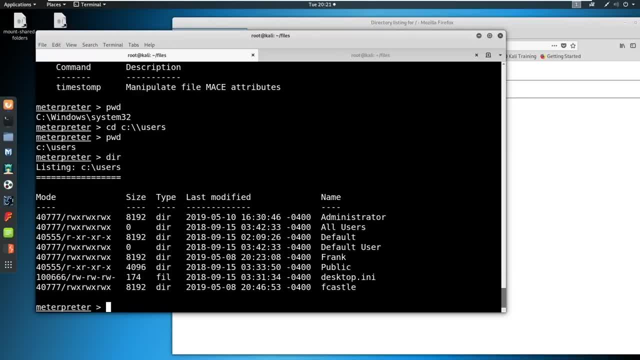 users folder. if we say dir. okay, there's a couple users. so what I want to do is I want to go to that area. I want to do is I want to. I want to upload the secrets file into this folder. so we're just gonna say upload secrets and you could do this. you know you could do this as. 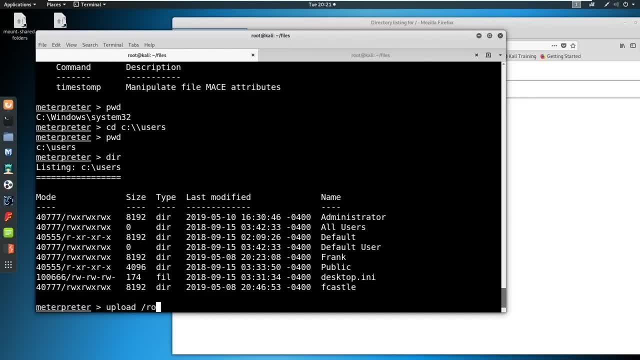 any file doesn't have to be in the directory you're in. you could say root, what do we put it? file secrets at text, something like that. and then if you want to put it in this folder, you would just say: secrets that text. or you could say: let's just put it in the C Drive, right? 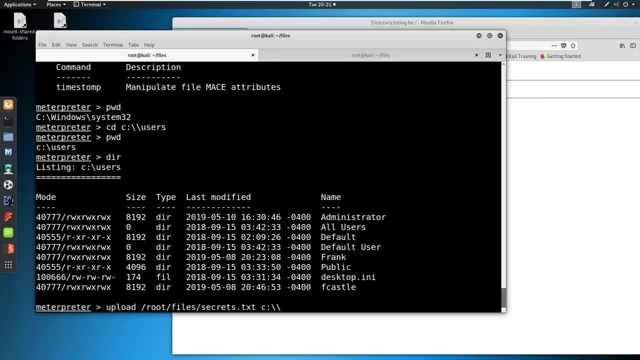 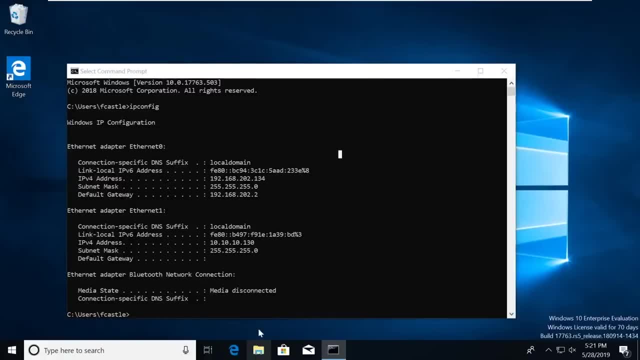 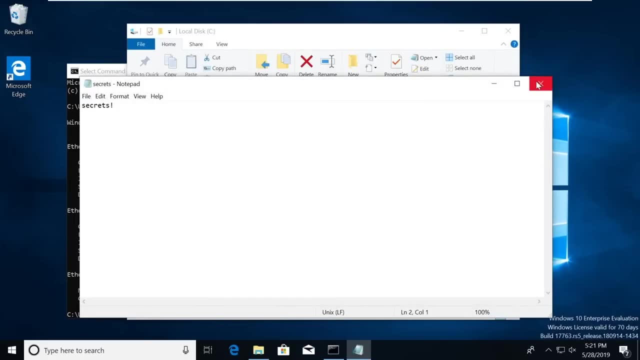 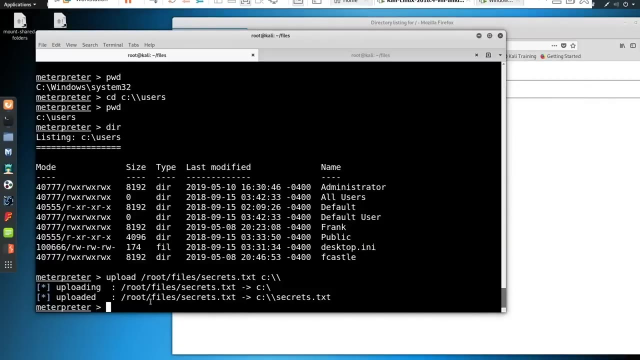 something like that. you just got to declare where you're putting the folder or the file and then it says it uploaded it to the c drive. let's go check out our c drive and there it is: secrets. so same concept. right, we can download that file and then we can go back to our. 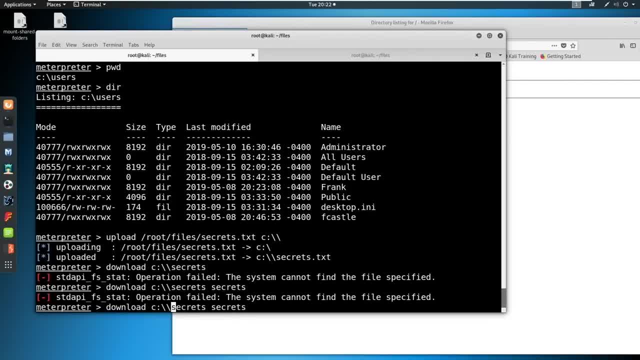 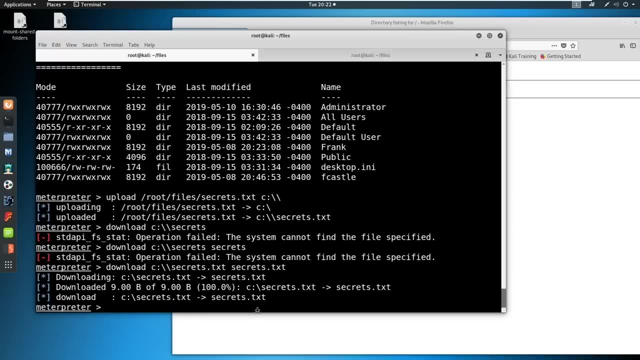 maybe, maybe not. oh, because i didn't declare dot text. i'm getting all fancy here. there you go, so we can also download the file and metasploit- one of the fastest ways. if you got a meterpreter shell, you might as well just use this to transfer your files and 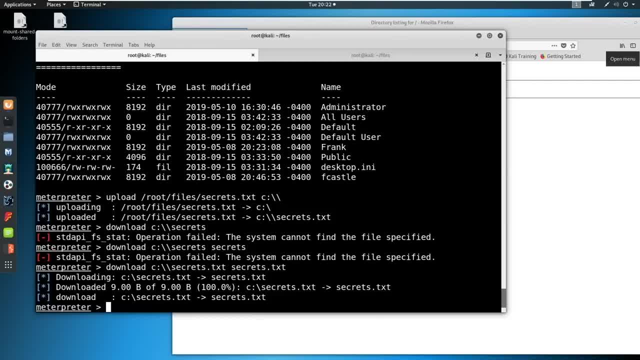 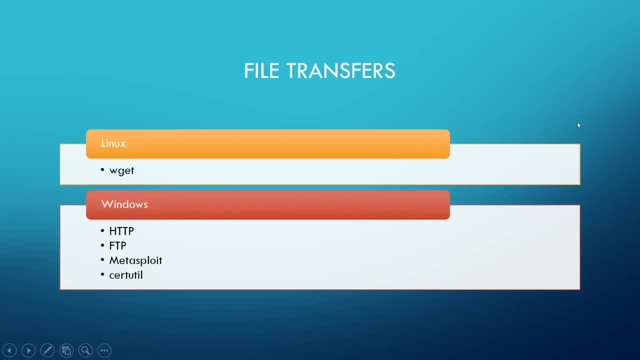 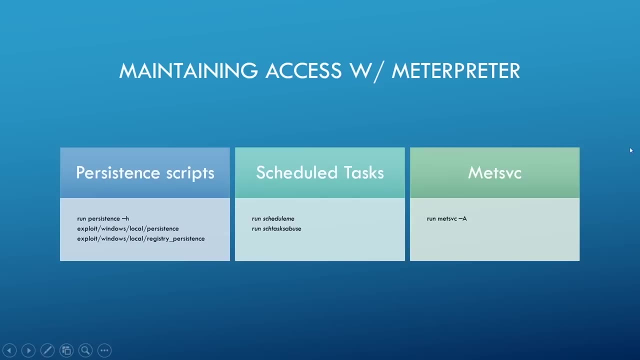 instead of doing it through a shell yourself- one of my absolute favorite ways. so while we are in metasploit, let's talk our next powerpoint section. so i put this in the wrong order, so let's go back and we're going to talk about maintaining access with meterpreter. so we've got a few different. 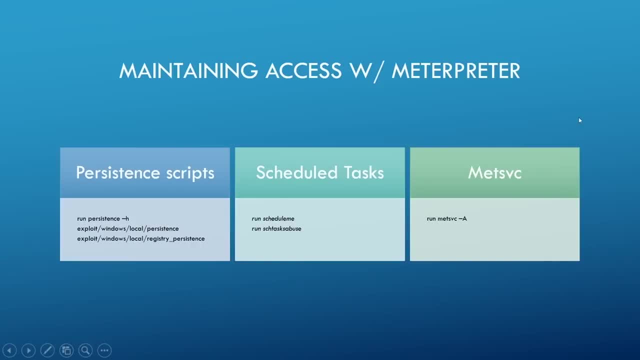 things i want to talk about. uh, we've got- these are all in meterpreter, like i said, we've got persistent scripts. we've got scheduled tasks. we've got uh met svc. now i'm not going to be showing you any of these tonight. these are. these are likely really not going to come up. 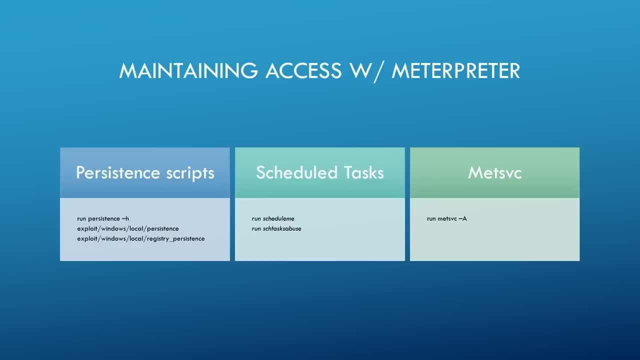 in a junior level pen test. i don't, honestly, i don't see persistence much um like, for example, the run persistence. i don't see persistence much like, for example, the run persistence. this dash h is just a dash help and i can show you that like we could talk about it. let's go back. 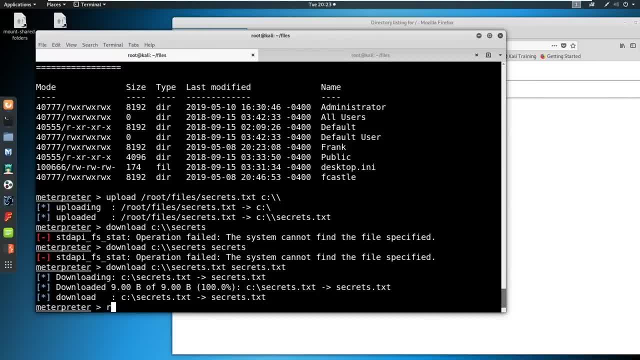 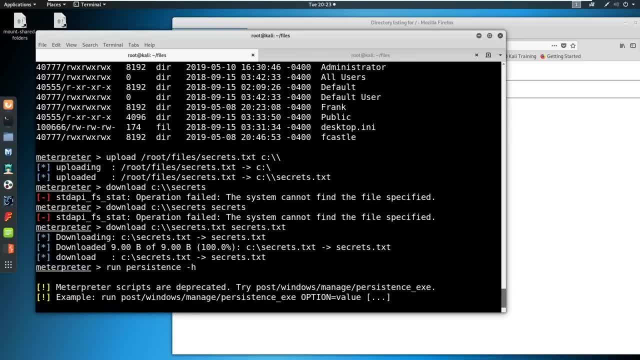 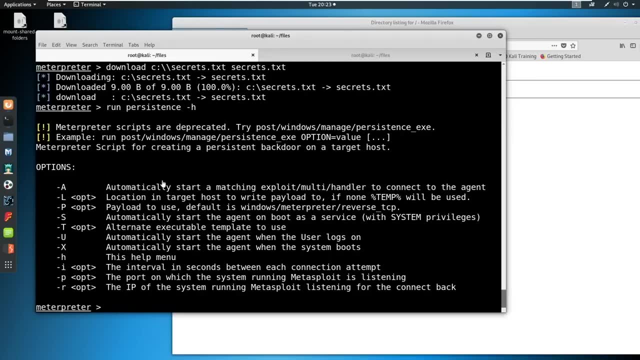 um, this is just like a really. it's like a really dangerous thing to run and you say dash h, like this, and so you have to declare all these values right, but what it does is okay. what options do i want? do i want to? um, do i want to automatically start an agent when it boots? 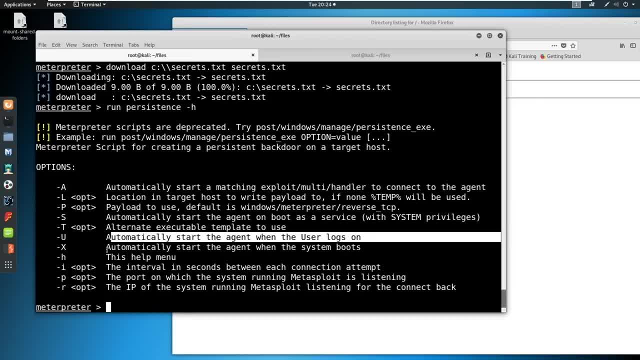 as a service. do i want to start an agent when the user logs in? do i want to start an agent when the system boots? what's the ip of the system that we're going to reach back to? what's our ip, our attacker ip? do i want to set a port right now? if you go and read the meta exploit documentation, you 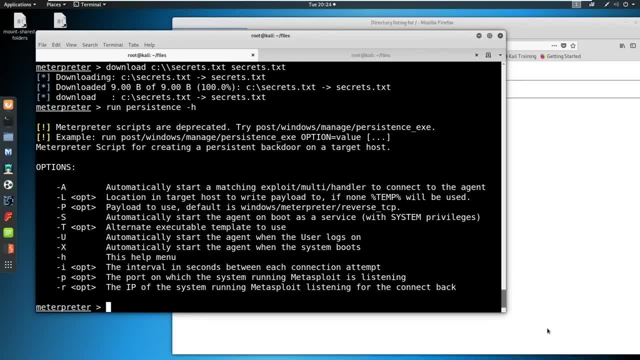 read metasploit unleashed, it tells you that this is a very, very dangerous module. to run that, really, as a a penetration tester, you don't need to be running the system to do that. you don't need to be to be running this unless you you absolutely need to. um, and the main reason is is it just opens up. 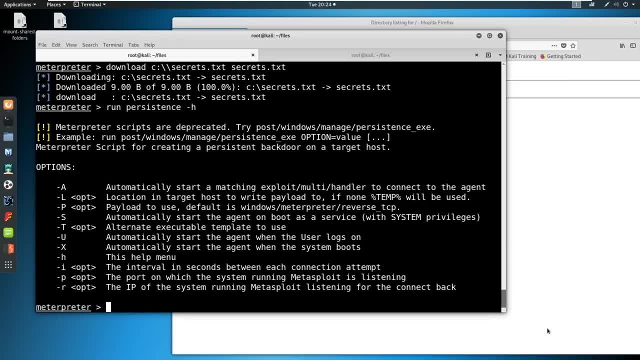 a port on a machine. that port doesn't have any credentials. you just basically connect back to it, right? so um, you're just leaving it wide open for a future attack and you actually have to go back in and delete the service. it does input it into the registry. you have to remove it from the 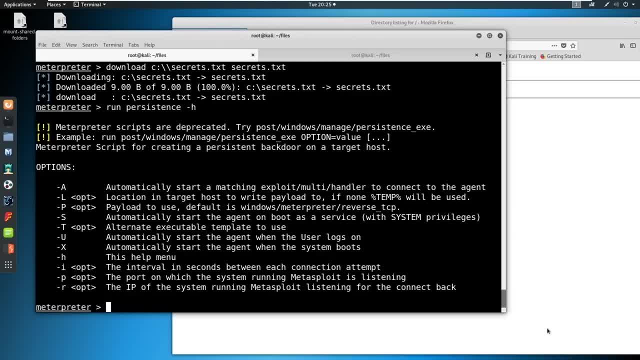 registry. this will give you an rc file, if you're connected, to go in and actually delete all those files for you. so it does have some cleanup, but but tools like this are dangerous and there's not a lot of need for them when it comes to- when it comes to, i would say, junior or mid-tier level pen. 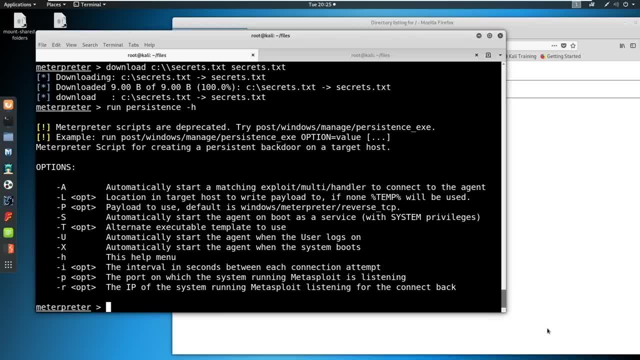 testing. if you're doing red teaming or something where you're being very, very discreet and you need a computer, you're on a host and you don't want to lose access to that host, that's a completely different situation. but when you're in a time, limited engagement, chances are you're not going. 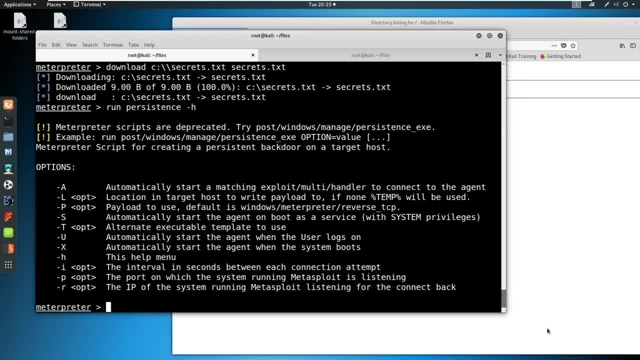 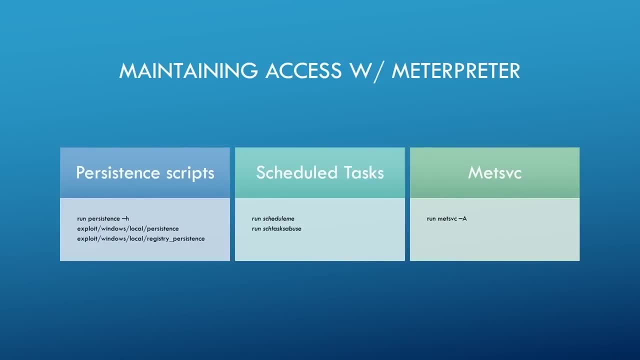 to ever need this. so i'm only going to show you the high levels for this. we're not going to go too deep into it because it's just going to be deeper than we need to go. so let's go back to the powerpoint so we can do it through persistent scripts. there's a few here. uh, exploit windows local. 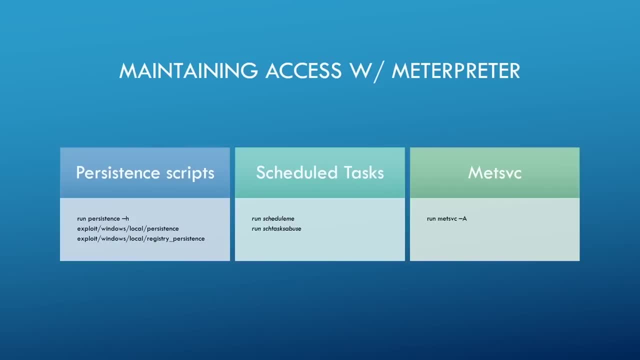 persistence is pretty close, if not the same thing, to this persistence. that's h. it just uh allows you to upload malware. there's actually some if you do a show advanced, it allows you to use your own executables instead. um, there's a registry persistence as well. there are scheduled tasks persistence, so that way. 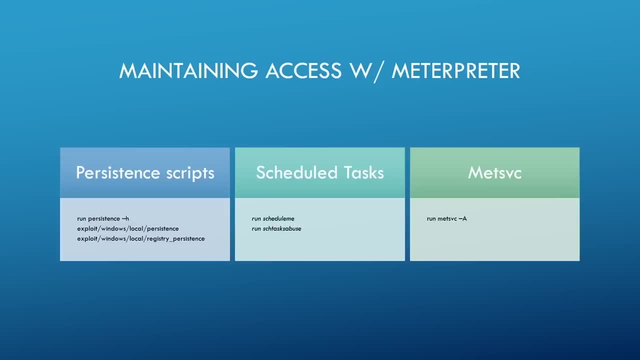 um, you can schedule a task basically to run the same time every day that runs your, your executable, so that way you gain a shell at least at some point, right, and you would just sit there with a listener. and we haven't actually covered the listeners. um, we haven't actually covered those. 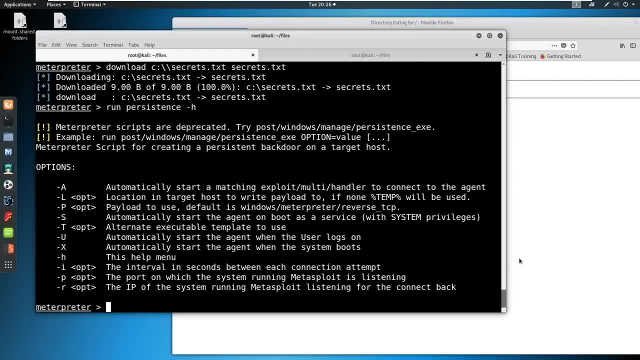 and i can show you what i mean by just a listener, so you could have like a netcat listener. but um, if you're trying to gain a meterpreter, shell back. let's just background this session that we've got so we can use something called exploit multi. 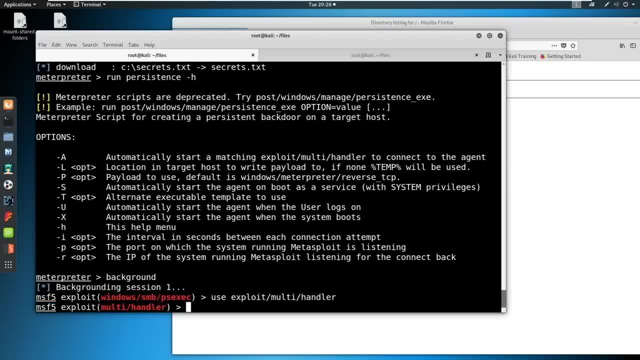 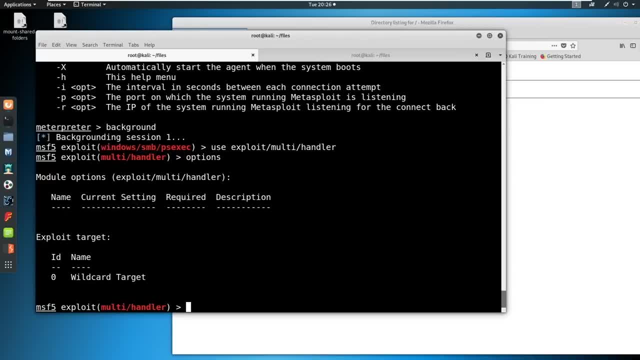 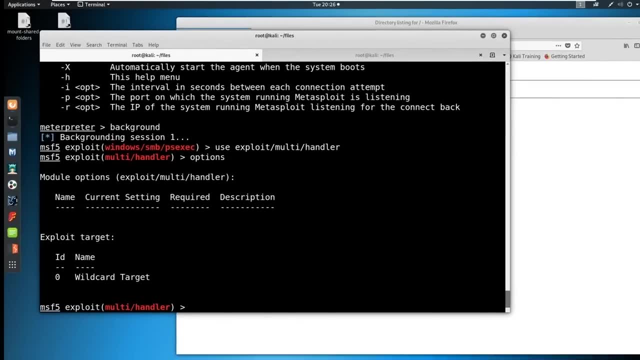 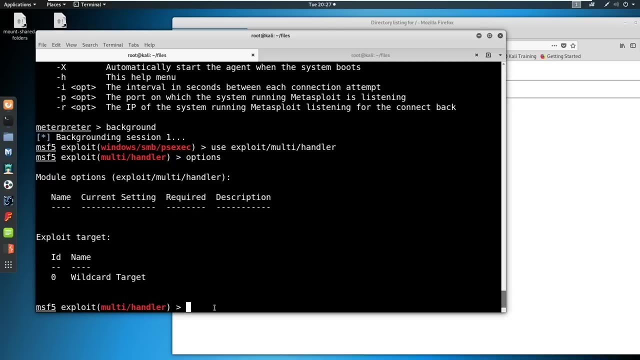 handler and if we say options on this, so it doesn't really show you what it does. um, oops, i moved my screen. i'm sorry guys, and it cannot go back there. we go. don't know if you saw that, but sorry, i clicked the wrong thing. um, so it really doesn't show you what it does here. but what we can do is we actually set. 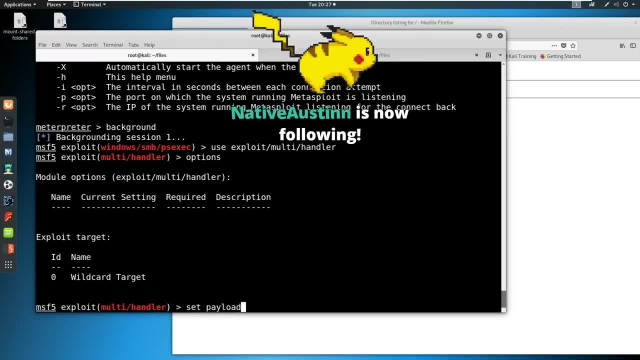 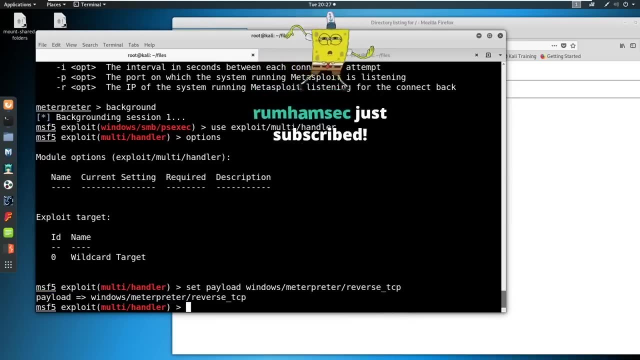 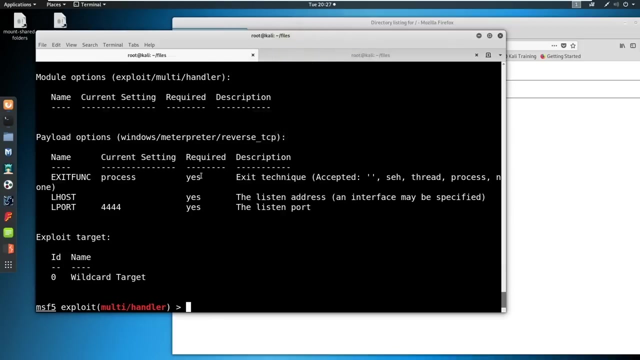 a payload. so we'll say, okay, the payload i'm going to be sending through this exploit um, is going to be a windows interpreter, uh, and we'll just say: reverse tcp. hey, thanks, matt, i appreciate that. and then you say options again. now you'll see that it it gave you this, uh, reverse tcp. you might set the l port to something sneaky. 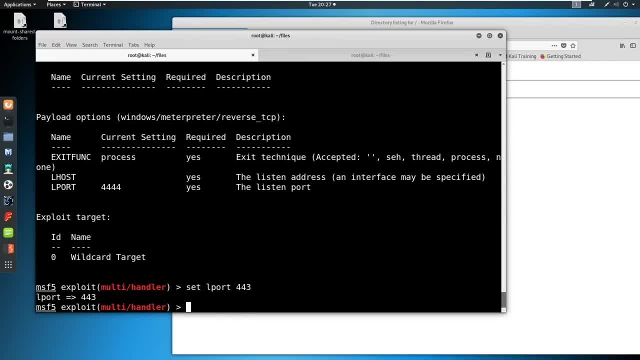 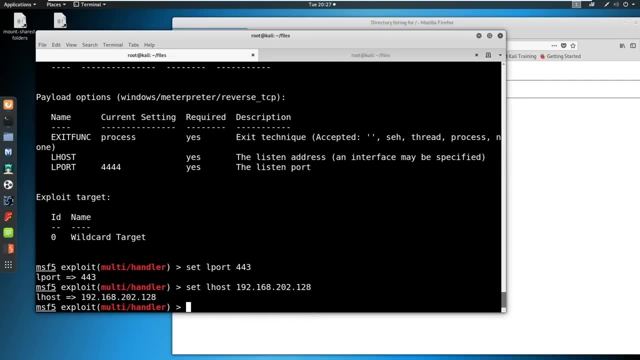 you might say: set l port to 443, so the traffic goes out on a known port, um, and then you would set your l host right, uh, whatever your ip address. so our rl host is um, 192, 168, 202.128. and then you would just say: run. now you can run this with a set of switches that'll put it in the 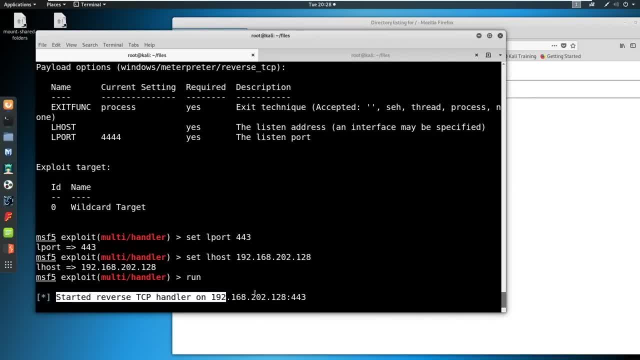 right place, and then you can run this with a set of switches that'll put it in the right place, but just just to get an example, all you're doing is running a handler. this is very similar to netcat, where you're listening- we're listening right now- on 443- for any traffic to come into. 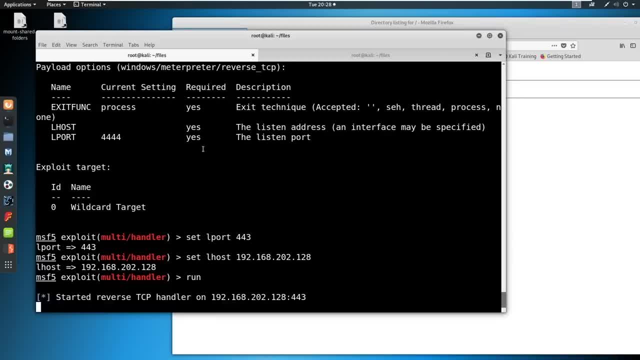 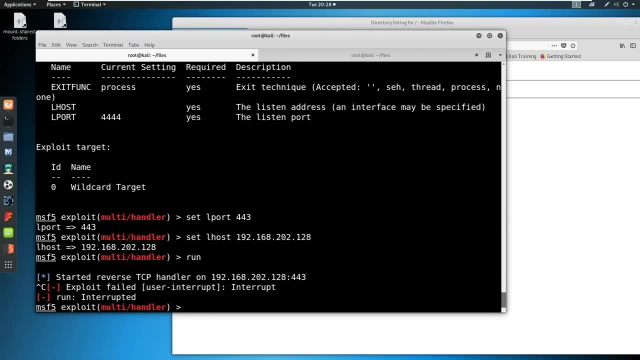 this ip address, um, and if it matches this payload, it'll talk back. it'll start up a meterpreter shell and that's how these persistent scripts run with the with malware. so, other than that, um, i encourage you to look into the these. if you want to play around with these, build your own lab, just note. 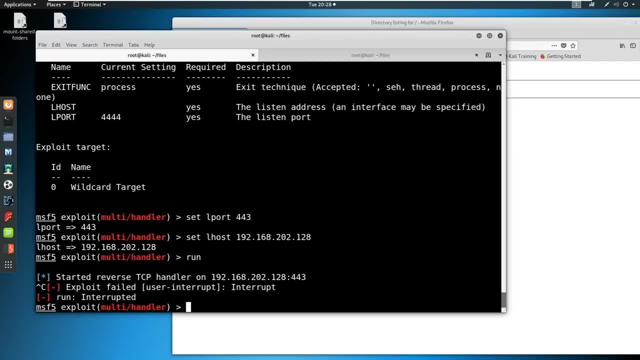 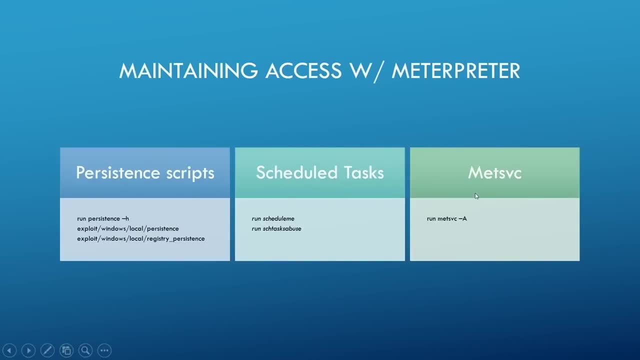 again that you're going to scrub the machines when you're done, because these do leave open ports, so make sure they're vms, or you are closing the registries and open ports when you are done, so going back in. you can also look into met svc, similar to the rest, another persistence module. 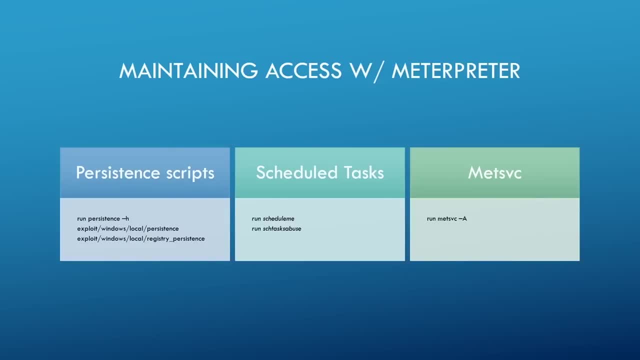 this is not all of them. there are actually a lot of persistence modules in meterpreter, but these are the generic ideas. you want access to come back to you if you lose it. if a machine like you have a laptop, you access and they take it offline because they go home. when they go back, you want to connect and talk back to you. 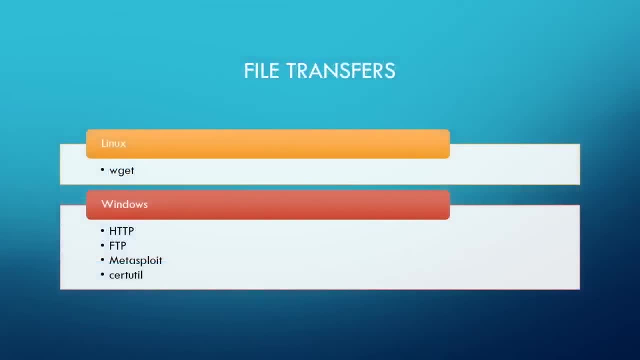 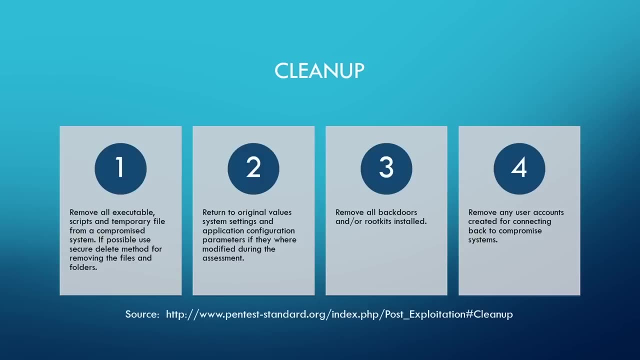 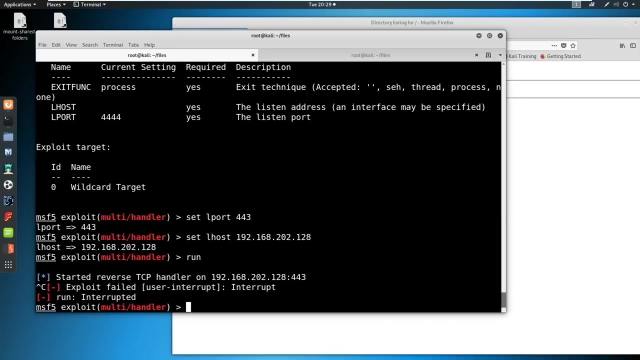 so that's the thought process. so what's up next? not cleanup, we're gonna go talk about pivoting. so let's talk about pivoting, okay. so we are going to do a pivoting lab together. we're going to build this out. i've already got. 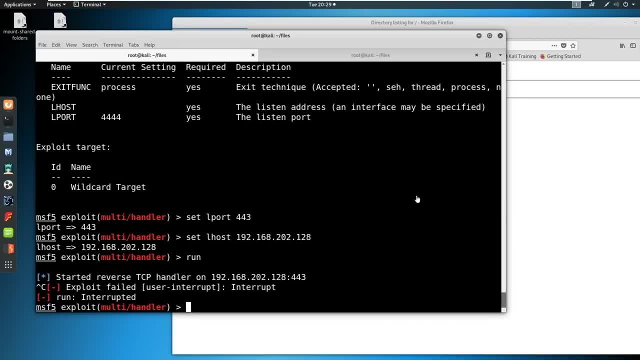 mine built out. so i will try to be as patient as possible- and i'm going to talk about pivoting and patient as i can be, and what we'll do is we will come into here and let's go into workstation up here and i want you guys to go to edit virtual network editor pivot- yeah, i wanted to. uh, i wanted. 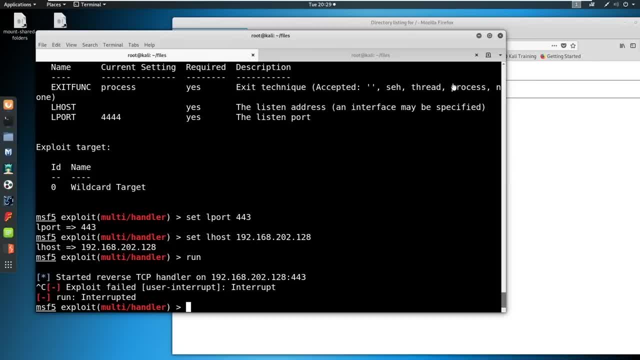 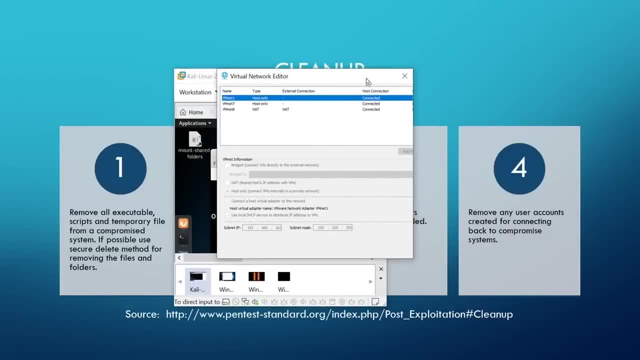 to use that in this, uh, in this talk, i guess, but i was afraid that i was going to get sued by friends or something along those lines. do i send the slides on discord? i don't ever send the slides out. um, i could. i don't actually think. 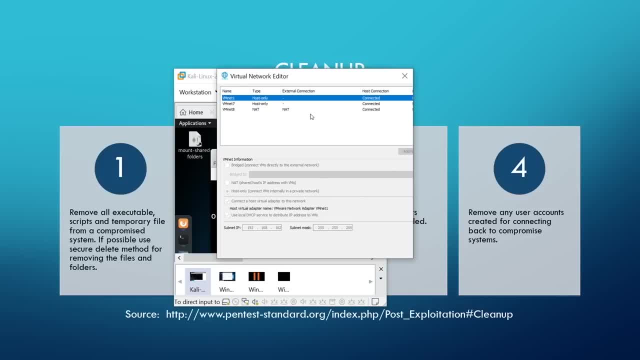 i have the slides saved. if i'm being honest with you, i've been running the same powerpoint, just deleting it, um. but you're more than welcome to take screenshots or whatever you like. um, so this is kind of hard to see and i don't understand why. what is going on? um, okay, so you? 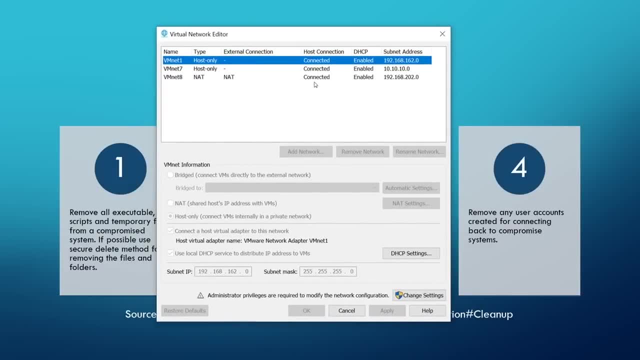 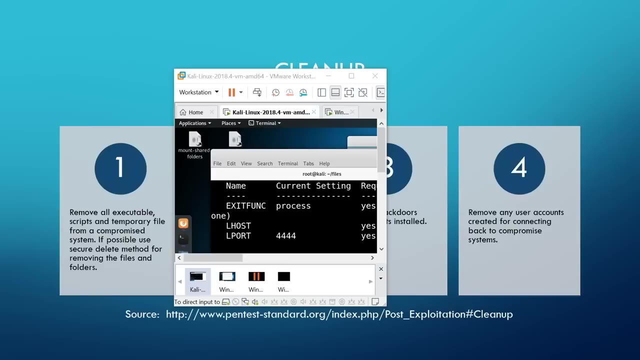 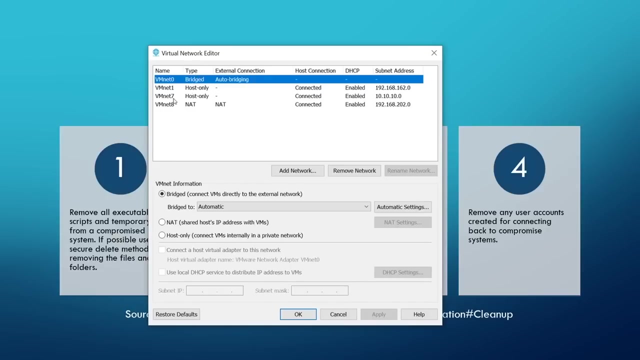 there we go. so you should see this, something like this: right, and you might just have a one and an eight here. i need you guys to go into change settings and that's an admin protocol. it's going to bring this back over again, okay, so you've got your auto bridging vmnet zero. you've also got um a one and eight. go ahead and 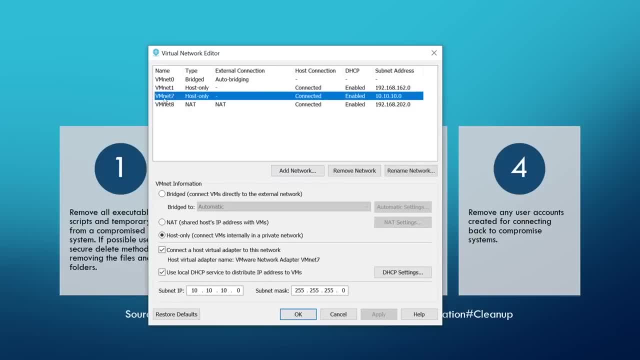 hit add network and i set it to vmnet seven. so look at my settings and i'll go slow as i can with this um. go ahead and select host only on these settings and then at the bottom, we're going to give it a completely different subnet. 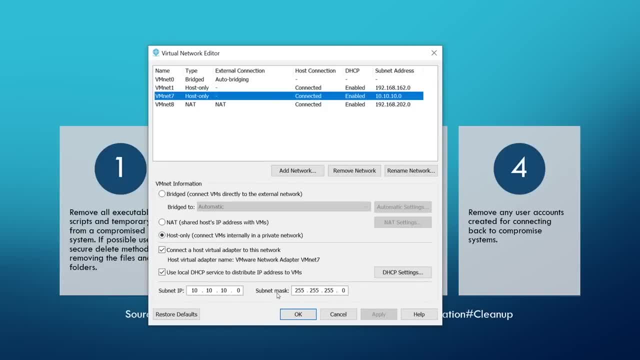 we're going to say 10.10.10.0 with a subnet mask of a whack 24, so all 255s with a zero at the end, and then you should have your typical one and an eight and an eight subnet mask, and then you should have your typical one and an eight subnet mask, and then you should have your typical one and an eight subnet mask. 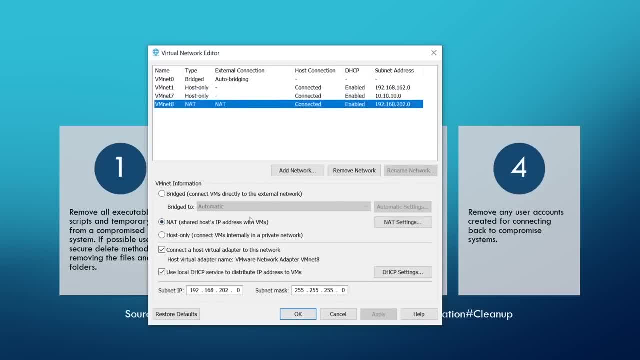 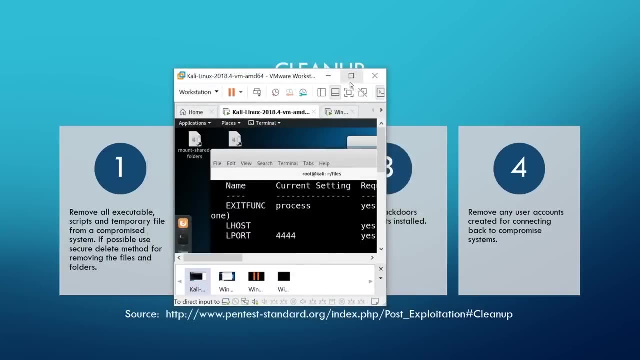 192, 168 down here with nat running um 202.0 is what i'm on, whatever you guys are on. however, you've been connecting. you want to use this guy here, so we're going to hit. okay, now we're going to have to do some things, some editing. 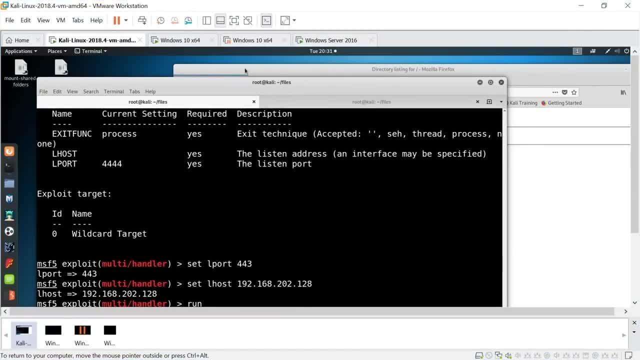 here's the situation, here's the scenario. let's set that up first. we are on a 192 network and we are attacking a- uh, a network. we've plugged into the network or gained access. we're attacking a network that is this 192 um, and we've gained access to a machine and we're going to gain access to a machine. 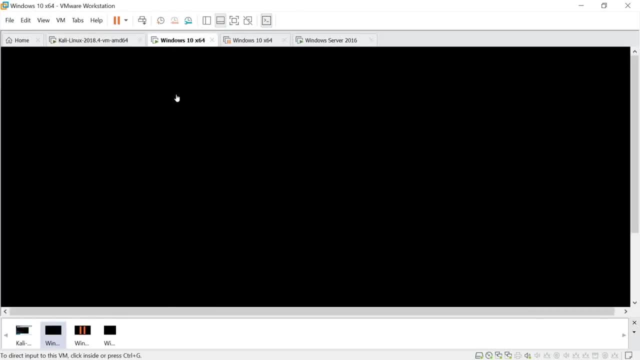 when we gain access to this machine, we realize through um, our enumeration, our post-exploitation enumeration, that it is a dual home machine, meaning that it's running on two different networks. so we see: okay, it's running on a 192 network and it's running on a 10.network. so we have until this time not been. 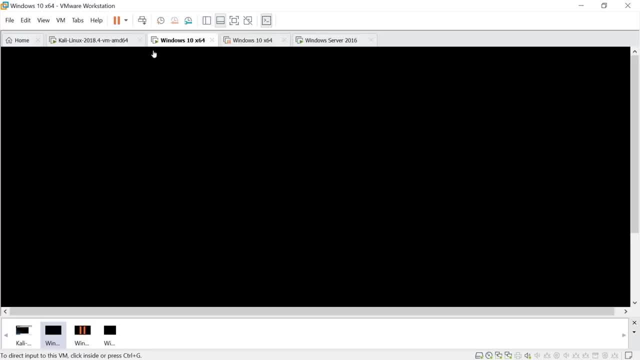 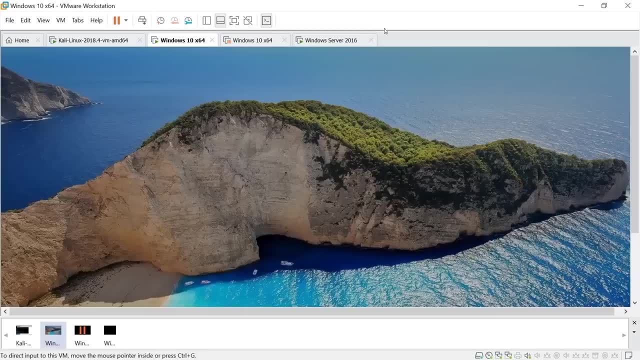 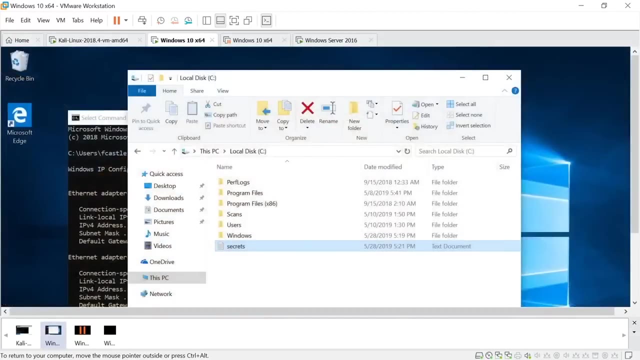 able to access that 10.network? um, we can only see the 192 network. so what i have done is i've set this up where our frank castle machine. if we come into frank castle um, he is running a dual home machine. and let me blow this up again: you go to the ip config, you. 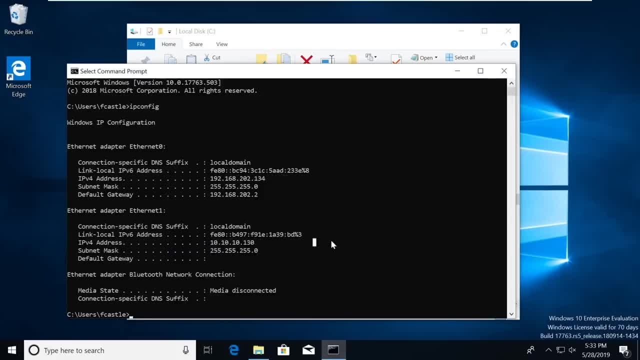 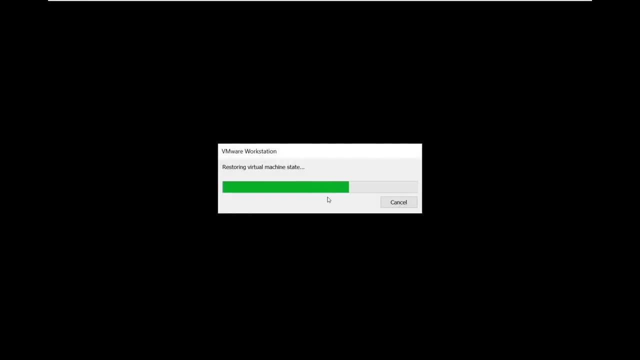 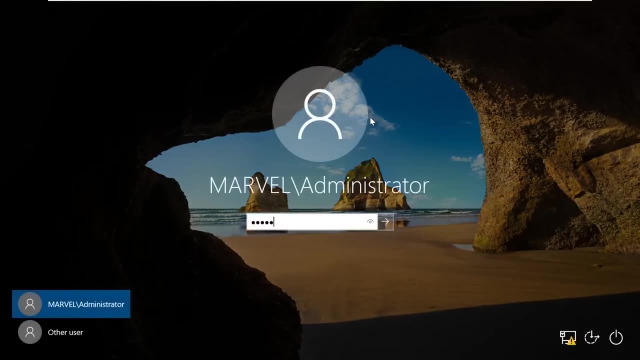 can see he's got a 192 address and a 10.10 address. now we've also got a peter parker machine that i'm going to power back on and i'm just going to log in as the administrator here two times the hot action that sounds sounds about right. 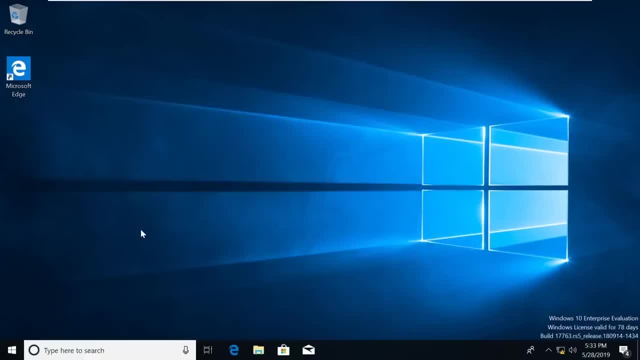 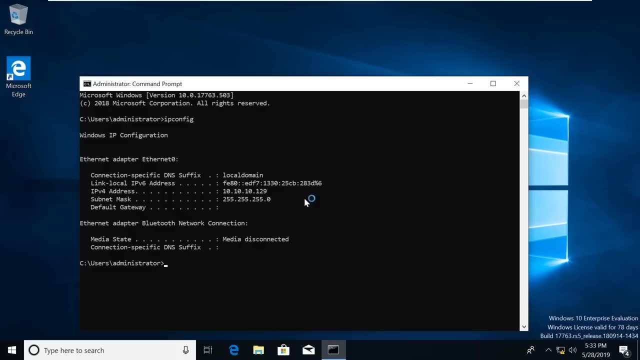 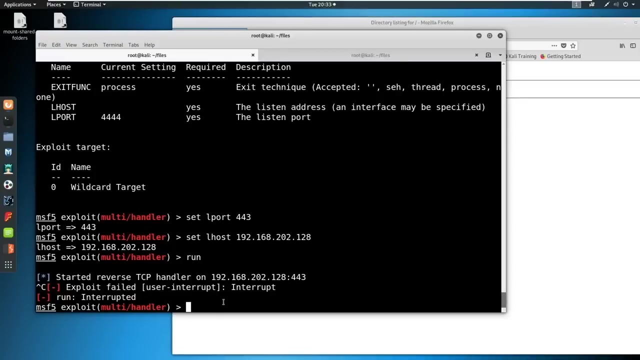 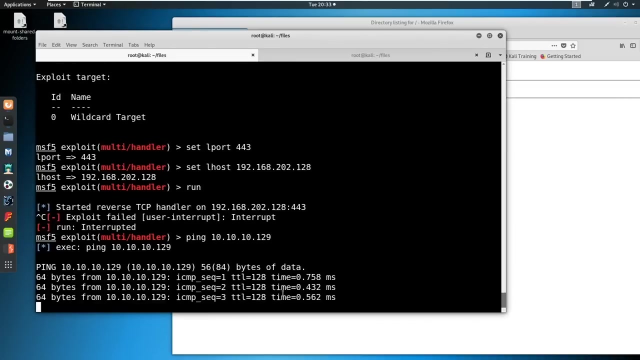 all right. we say command ip, config 10.10.10.129. so these two machines, they can talk right, but with this machine we won't be able to talk. we say ping okay, well, it should be able to talk right, but we're not going to be able to talk. 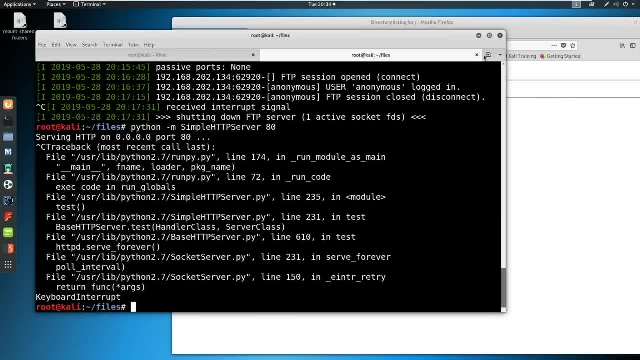 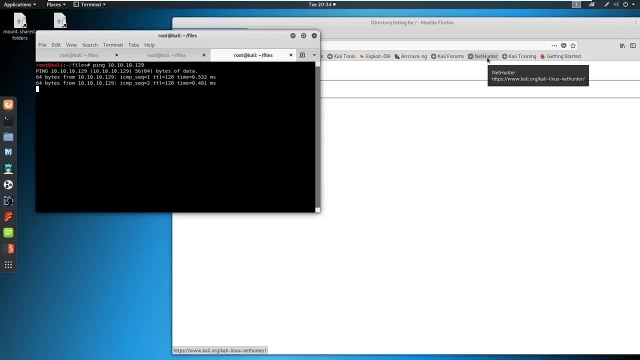 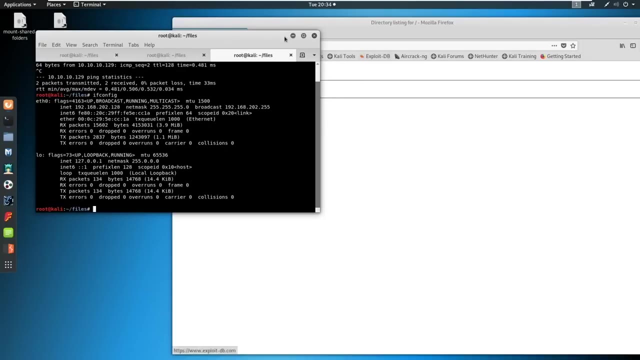 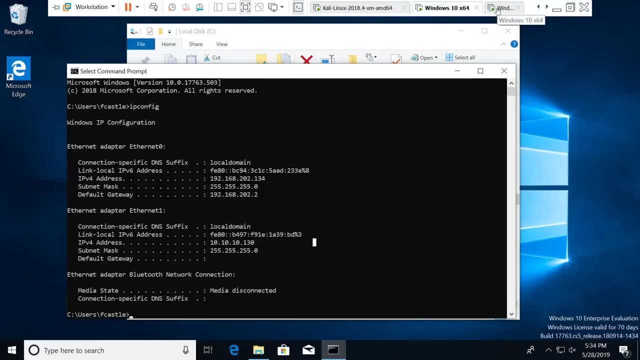 it's talking through. it's talking through metasploit- i got ahead of myself, sorry- or it's just talking. i don't know what's going on. it hates me, um. okay, no idea why they're talking. should not be talking, guys. so if we um, if we go in here, this is on its own network, right? 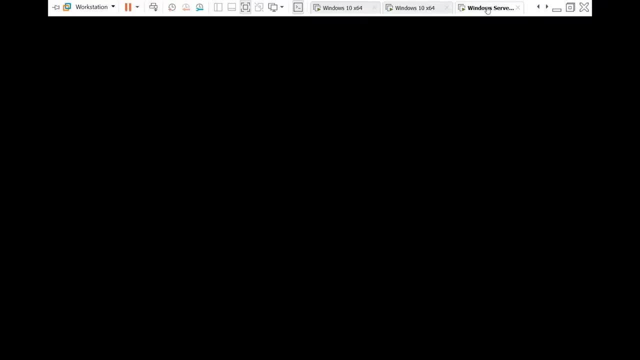 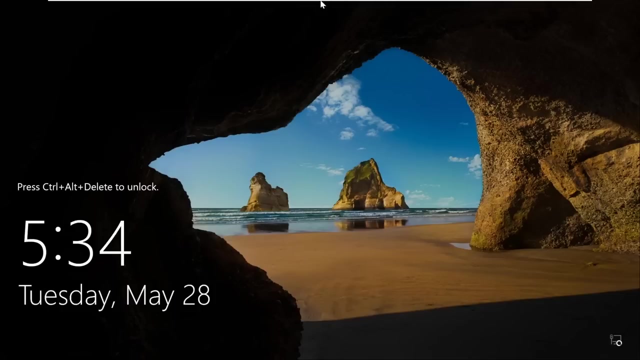 and the domain controller is also on two networks. let's take a look if i can get out of this screen now. it's not letting me. i am so frozen right now, guys, i don't even know what to do. let's see can i come back, all right? 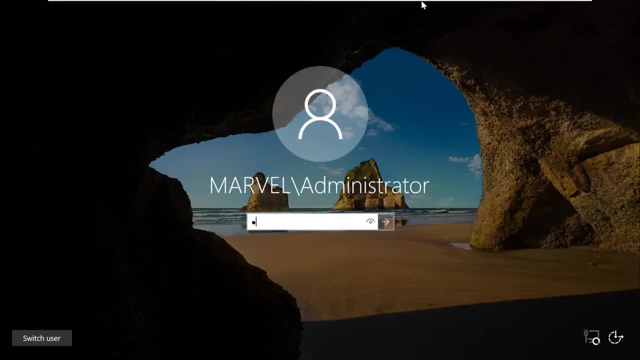 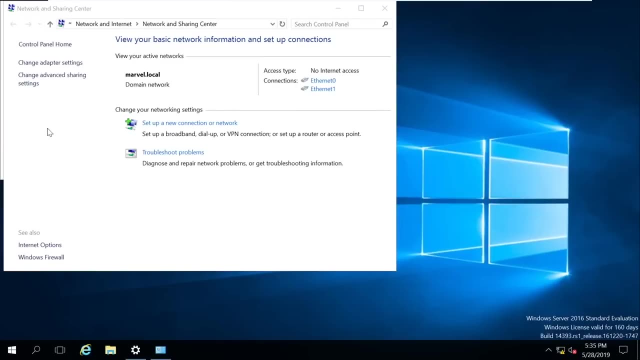 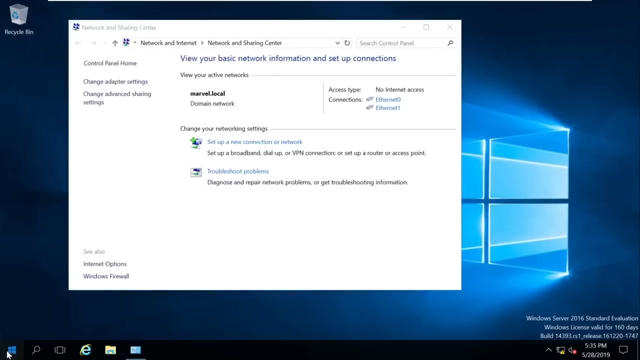 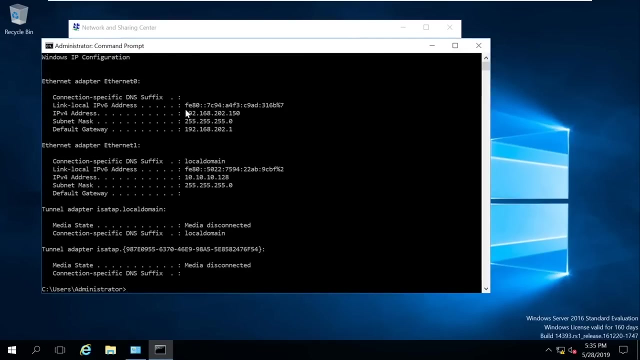 there we go: okay, okay, so, so, so, okay, so, so, so, so do that, so, okay, so do that. so If we come into here and we say command, you can see that we're running on 192 and we're also running to a 10.10.10.128.. 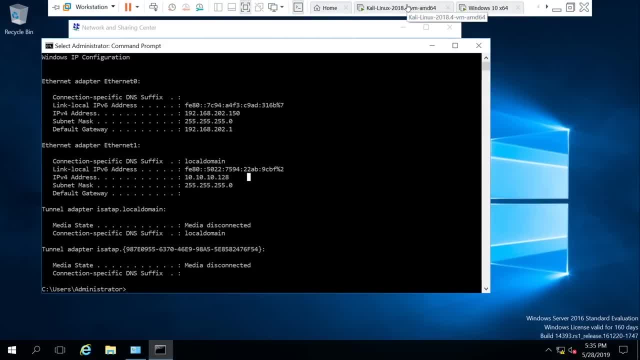 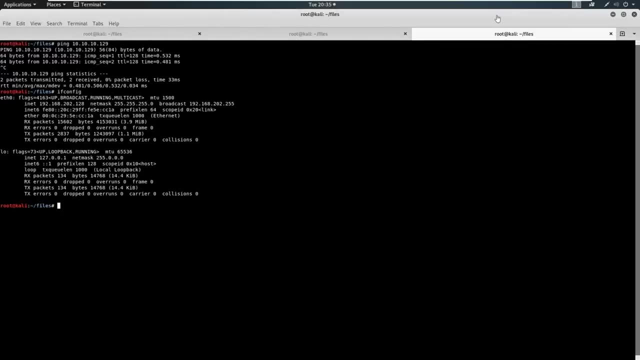 Now let's talk about the lab setup And you guys. in theory it should not talk for you. I've been doing a lot of pivoting the last couple days, So maybe there's something that got set up, some routing table that got configured. 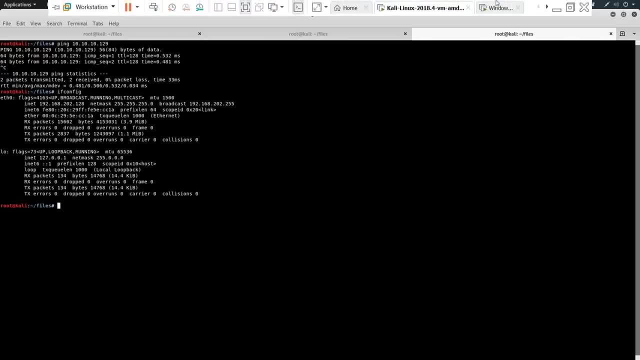 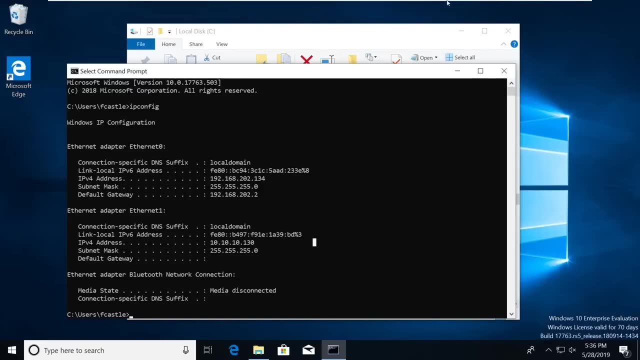 I did do an auto route with my meterpreter and it may have set a routing table for me, So I'm not sure the reason. Anyway, let's set this up. You're going to have to shut down all of these, So what we're going to do is we're going to shut down all the machines. 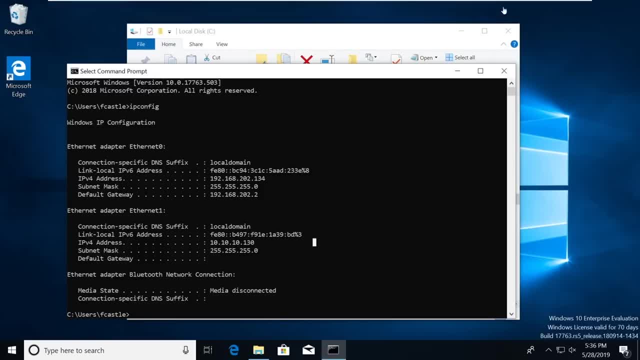 And I'm just going to leave mine on and running, But go ahead and shut yours down For your machine that we just exploited, the Frank Castle machine. what you're going to do is you're going to go into And you're going to- actually I'll pause it so I can show you. 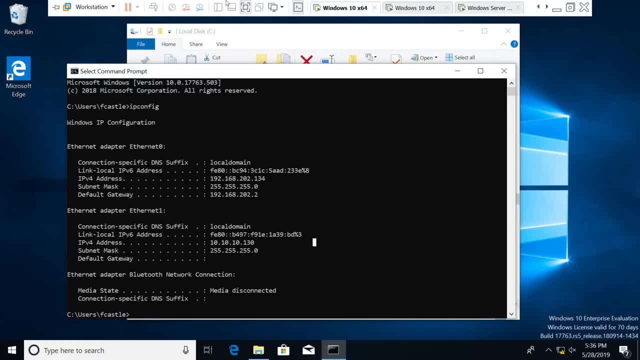 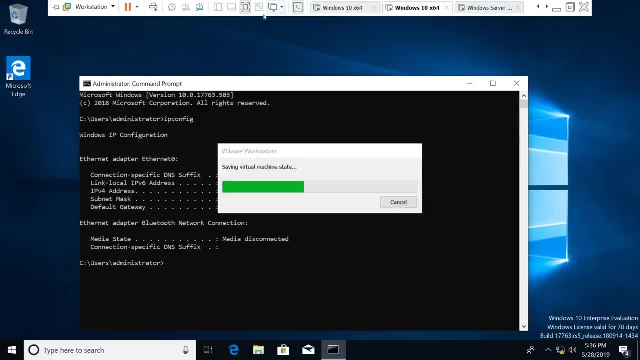 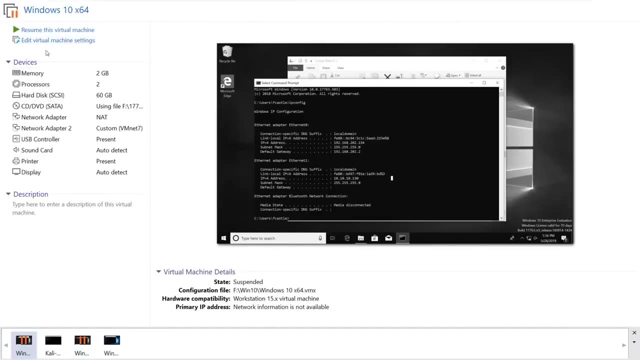 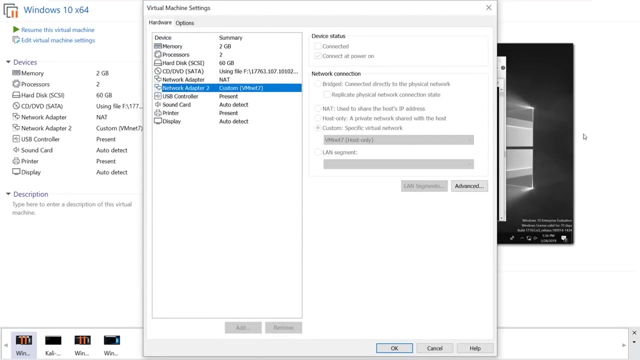 In your shutdown state. we're going to edit the networks And I'll pause all of these so I can show you. Okay, so if we edit the virtual machine settings, I won't be able to do this because I am- I am still powered on technically, just because I'm on pause. 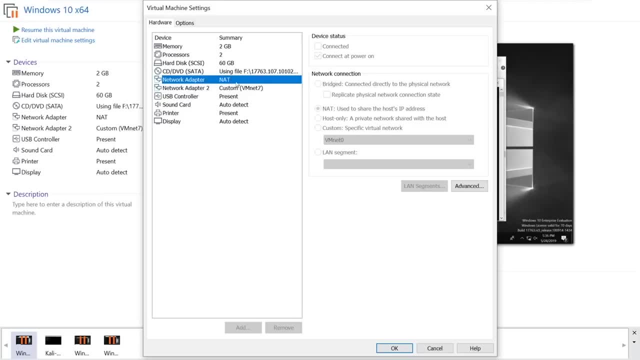 I have one network adapter on Frank Castle that is running NAT. I've got another network adapter that is running VMNet 7.. Remember, that's the second NIC, right? So Frank Castle is going to have two NICs. And then we come over to Peter Parker. 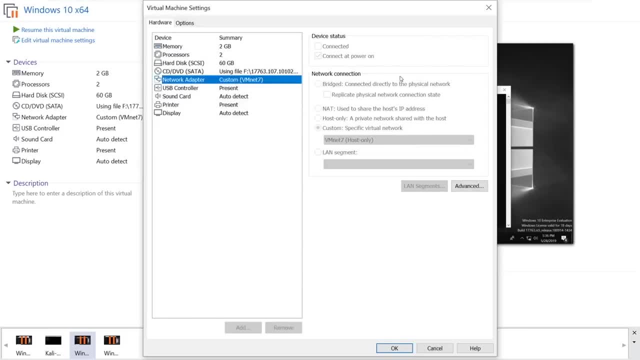 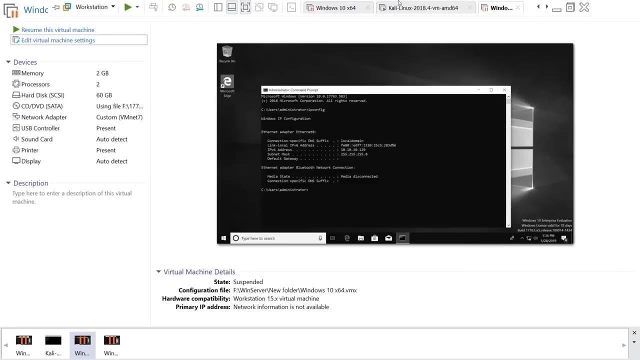 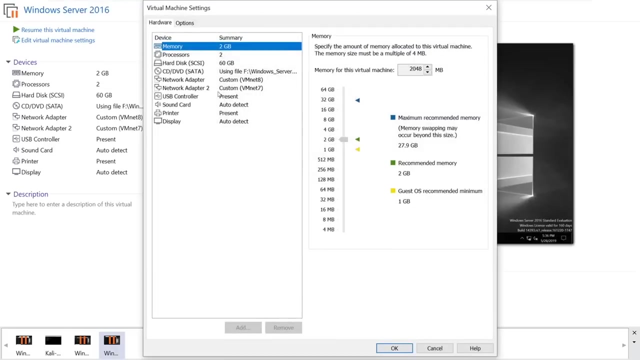 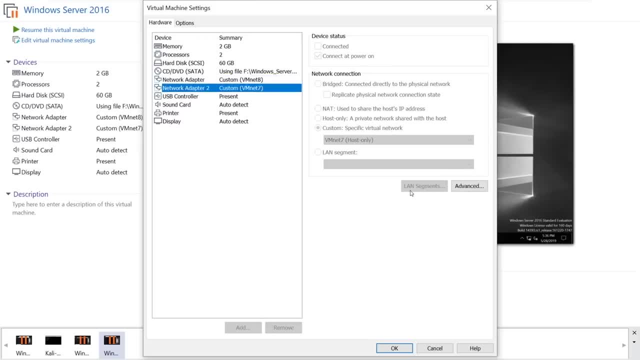 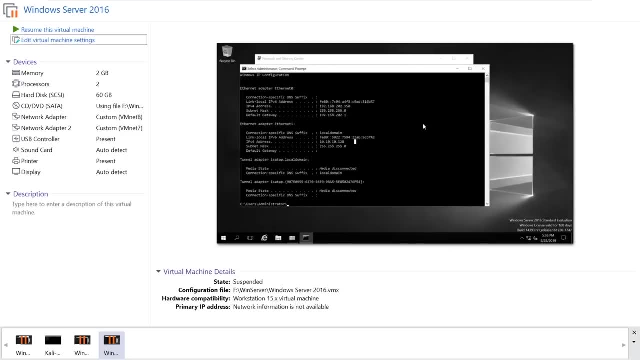 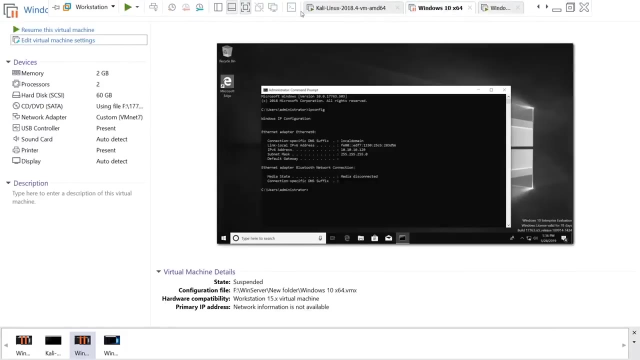 It's the same thing as NAT, VMNet 8, VMNet 7.. So two separate NICs. So go ahead and configure those. I'm going to resume these real quick And maybe troubleshoot why these machines can talk Okay. 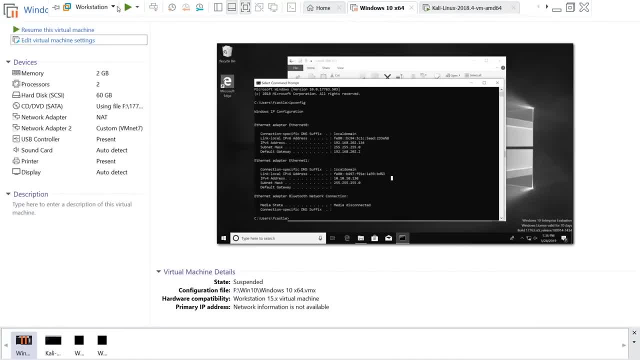 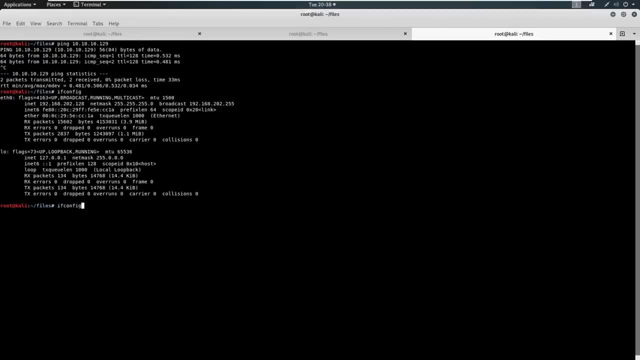 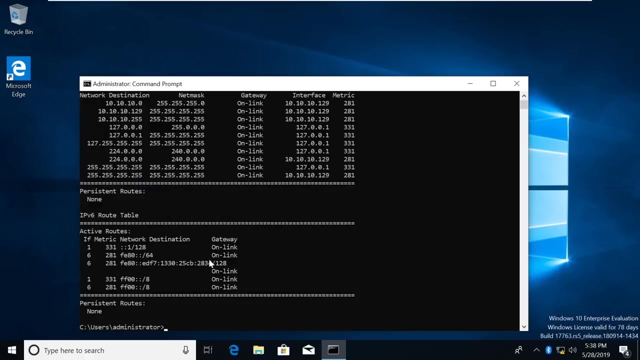 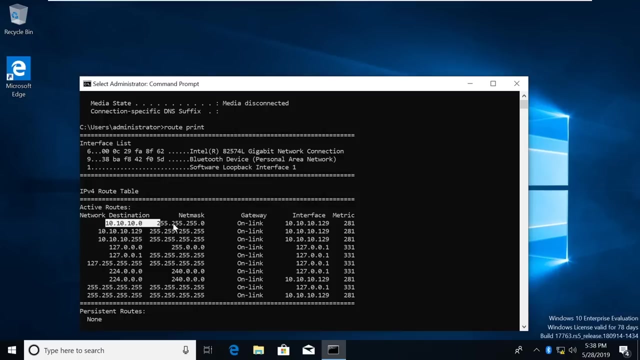 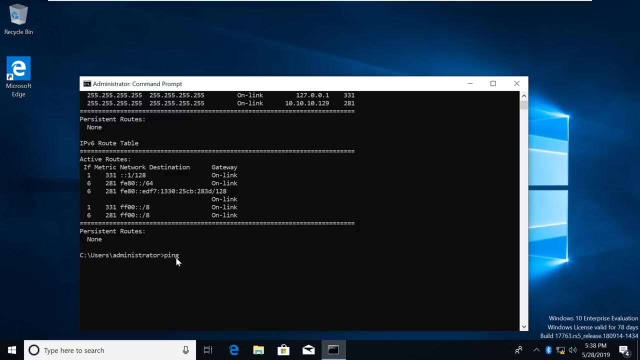 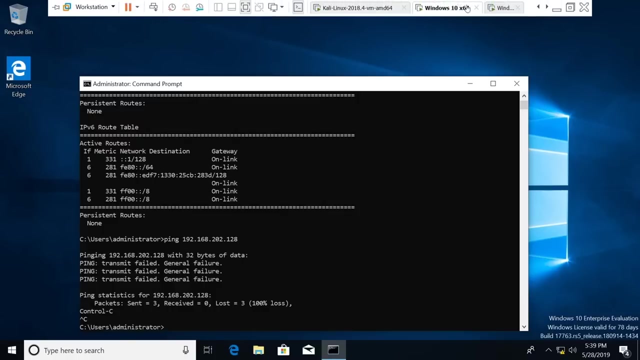 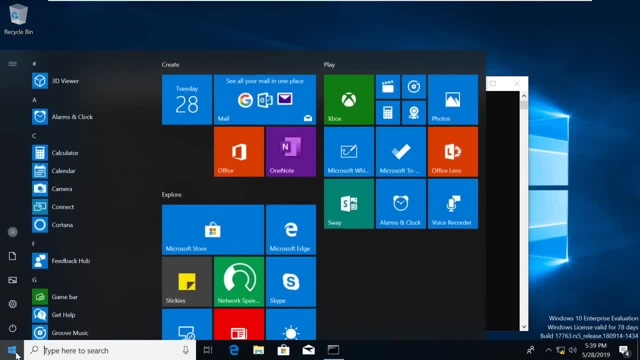 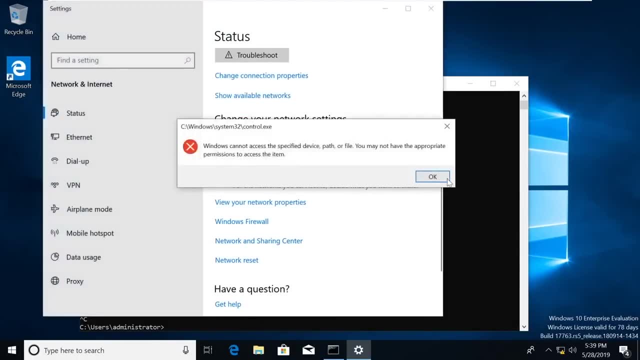 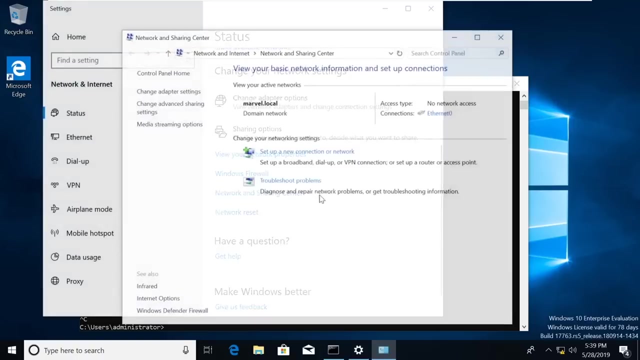 is if we come into the network adapter for Peter Parker. I'm just going to go into network status and then change adapter options. Okay, we'll go. Let's see Network and sharing center. Since it wants To be rude, we'll do it that way. 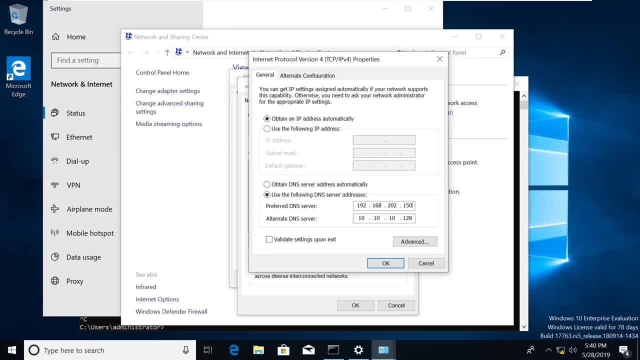 We have two. This has changed, The only reason I'm changing this. So I've got the preferred DNS for 192.168.202.150 and then alternate DNS of 10.10.10.128.. Those should line up with here: 202.150 and then 128,. 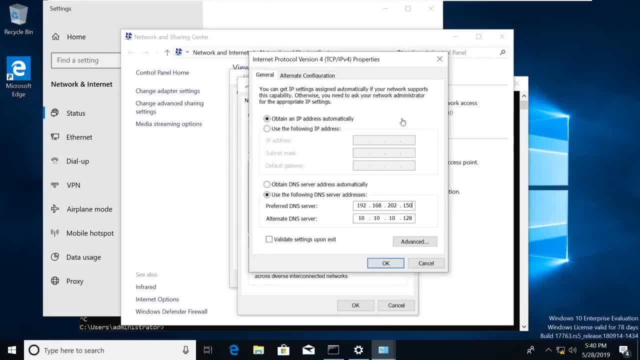 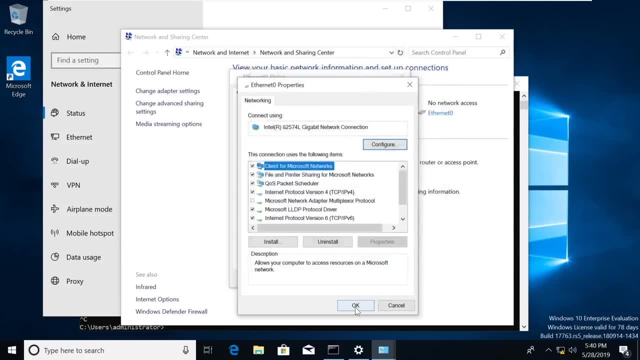 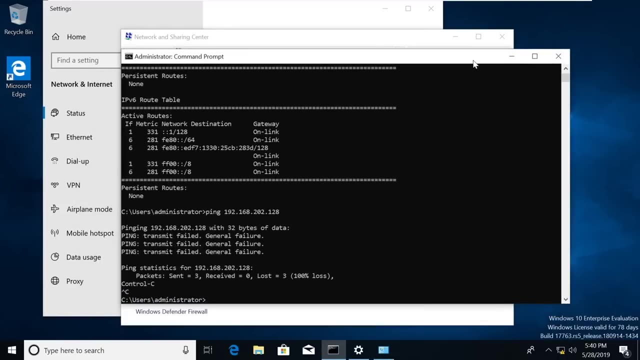 just so it's talking, And if it fails over, it's still talking. It's not connected to the Internet because it's not connected to anything available to be connected to the Internet. Second of mine, It doesn't have to be connected to the Internet. 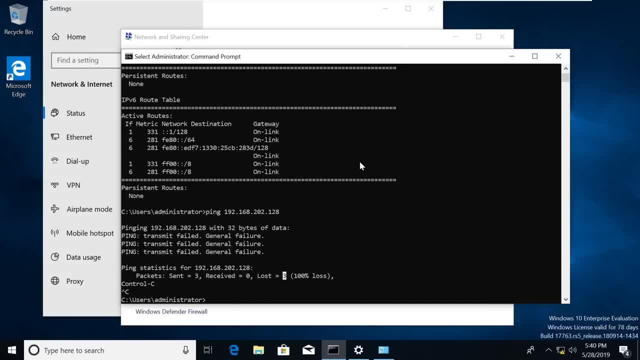 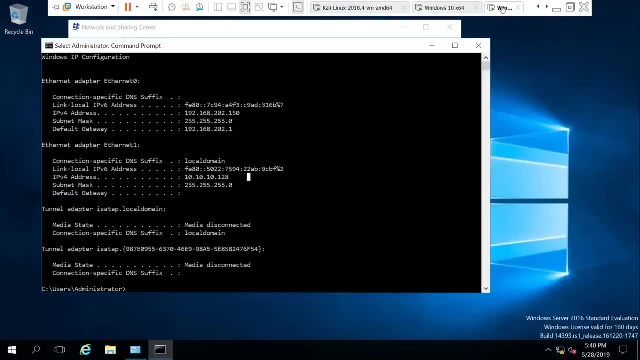 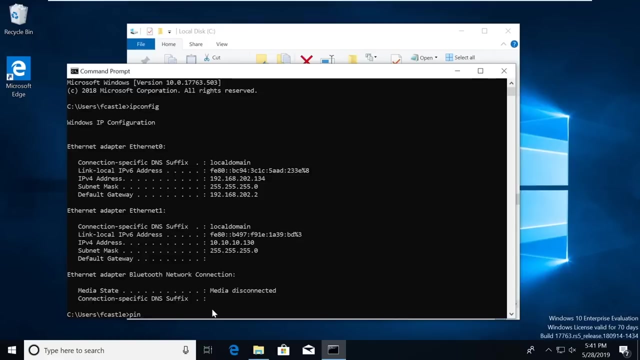 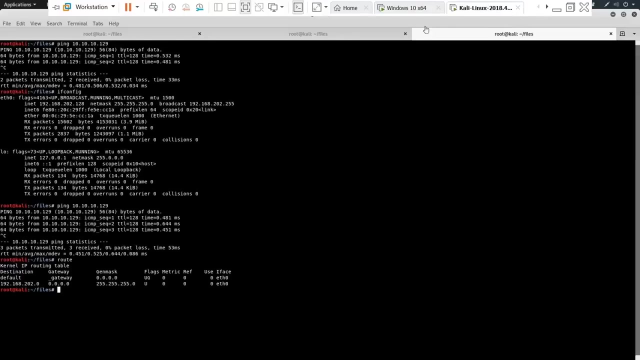 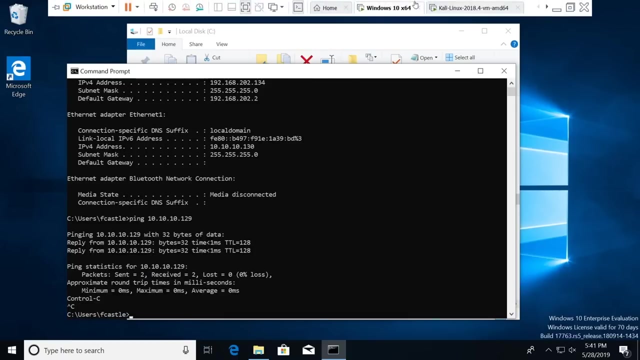 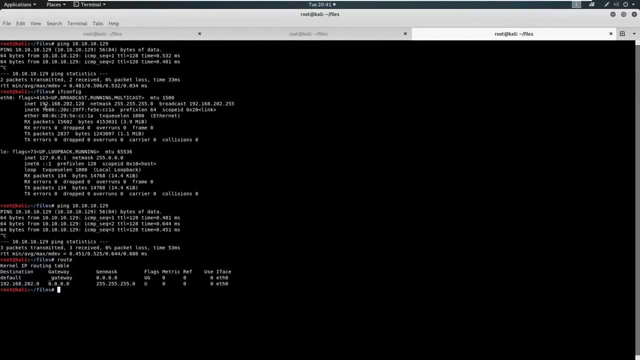 For this lab to work. What's important is that we can ping from our Windows 10 is that we can ping the other machine, So 129.. What I'm troubleshooting, Sick of the mind, is why my Cali machine that is sitting on a 192 network is able to talk out to a 10 network that it shouldn't know what it is. 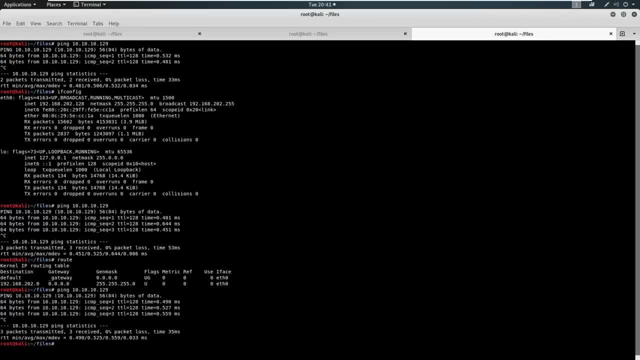 This should not be happening right, And earlier it wasn't happening. So I'm guessing that I have some sort of route that it learned and It can't talk back the other way, but it can definitely talk forward, So I'm not gonna worry about it. 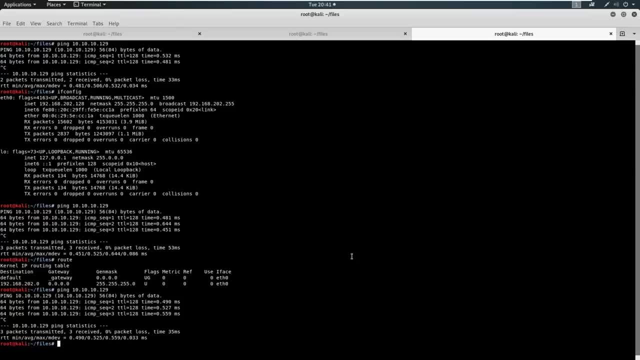 I'm not gonna worry about it. the lab, The lab will hold up for its purpose. guys, All right, how are we doing on the resets? If you're following along, Have you reset everything? Are you back up and running? I know this is a little bit procedure, I just didn't want to have to show all of it. classic demo problems: Absolutely. 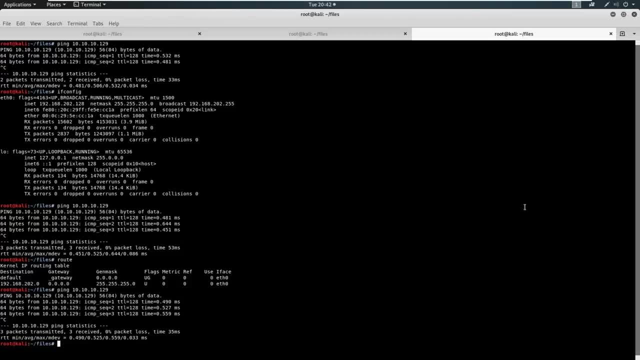 I know this is a little bit procedure, I just didn't want to have to show all of it. classic demo problems: Absolutely All right, we're gonna run the service networking restart, that we're saying. All right, we're gonna run the service networking restart. that we're saying. 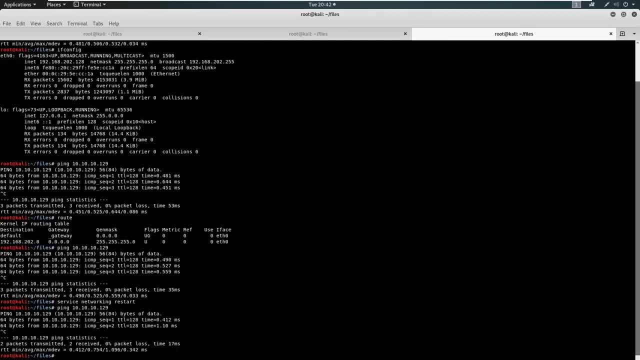 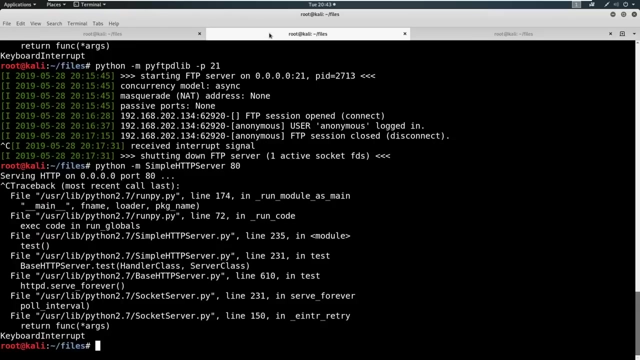 Still pinging, Still pinging. It's fine guys, I'm not gonna be too worried about it. So let's continue on. so we'll pretend, happily, that we are unable to talk to that machine. What we have is Access to a machine in Materpreter. Access to a machine in Materpreter. 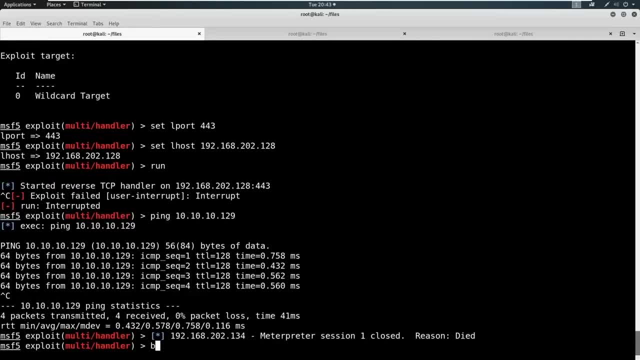 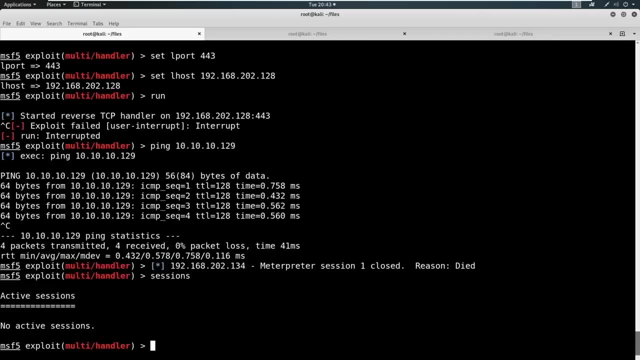 Access to a machine in Materpreter. So let's actually Background. Let's go to sessions. We have no active sessions, we lost it never mind, so let's gain our session back. So let's go to use exploit. Windows SME PS Exec. Windows SME PS Exec. 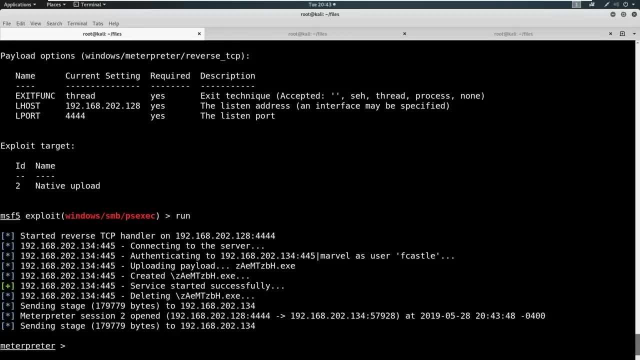 Options- just to make sure we're all the same, Let's try running it. Options: just to make sure we're all the same, Let's try running it. Okay, Now we can try some pivoting commands. we can first look. I'm actually curious. Let's look at the routing table if we've already got some sort of auto route. 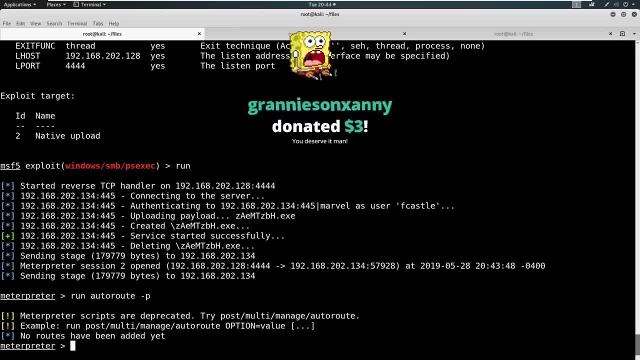 No routes have been added yet. so Hey, thanks, Grayson, I appreciate that. So we've got no auto routes. but what we can do here is we can say run auto route And then do a dash s and then we want to connect to that 10 network, right? so we're gonna say slash 24. 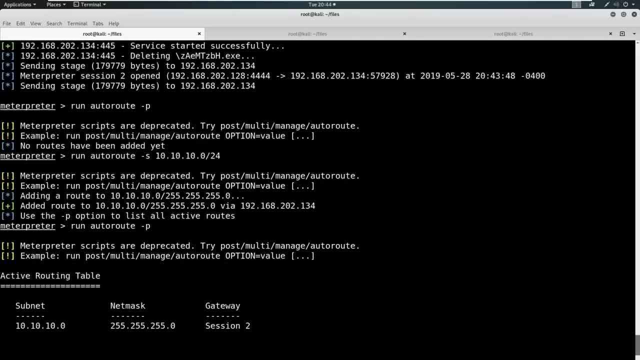 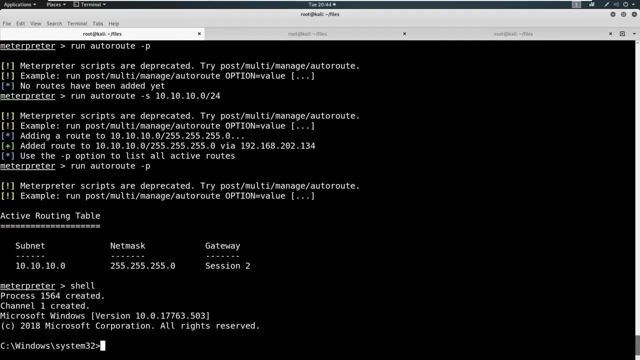 Okay now if we run the command again, You'll see we have a route in there through session two. So If we go- actually I want to show you if we go into a shell real quick. so some things to note, right. so if I am a 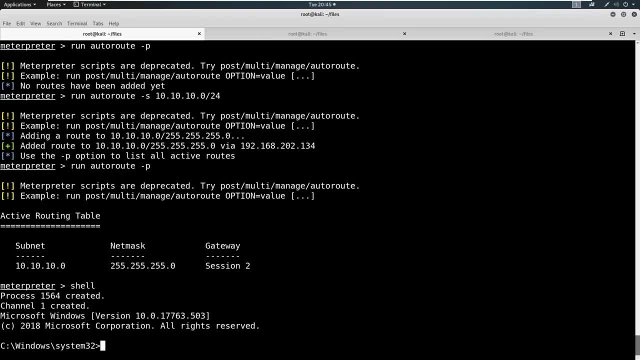 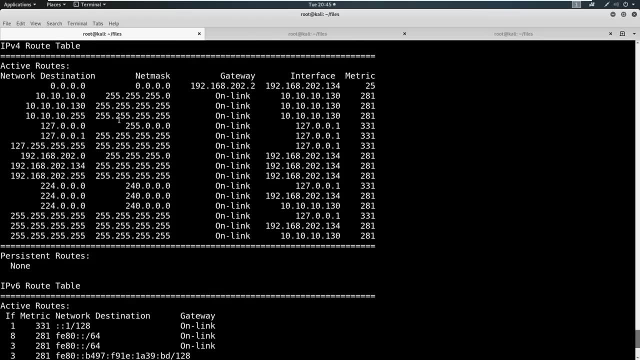 attacker an attacker. I want to see if a machines dual home. a couple things we can do is we could say route print And we can look at the routing table right and the routing table shows us that there's a 10 network And there's a 192 network. 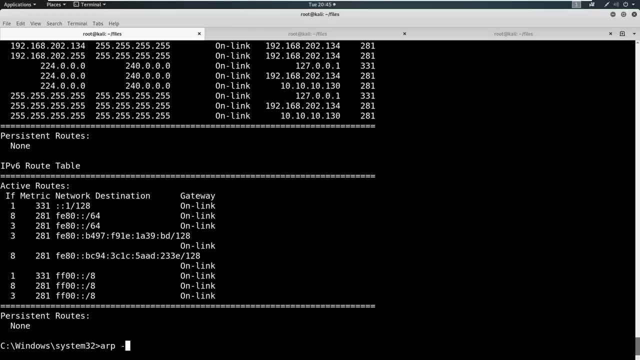 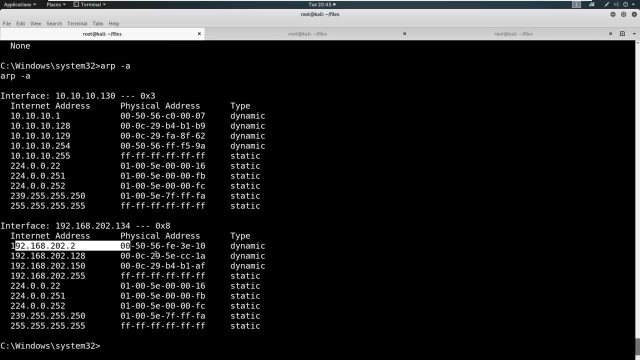 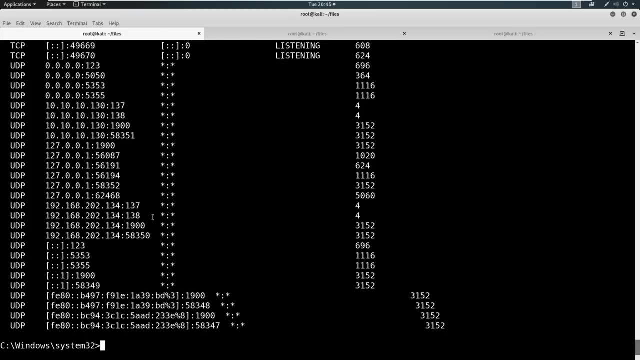 So that would be an indicator. You could also look at the ARP dash a and see the ARP table, And you can see that there's a 10 network in here and there's a 192 network as well. A net stat might show us some things if there's any communication between the 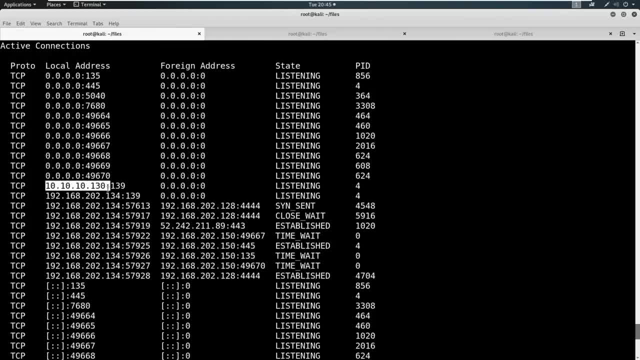 The two if they're, if they're talking over something. you can see a 10 here and a 192 here as well. We can see where it's established. You know some connections talking out here on 443. So sometimes in lab settings they've got a. 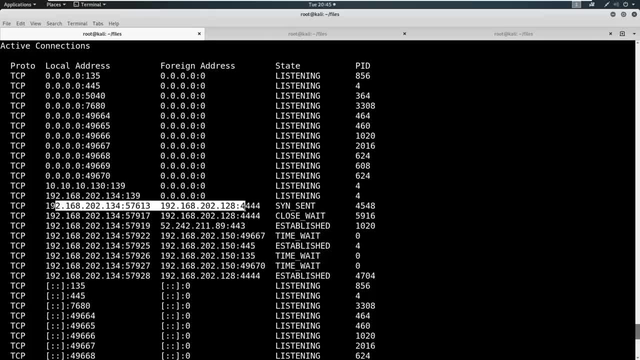 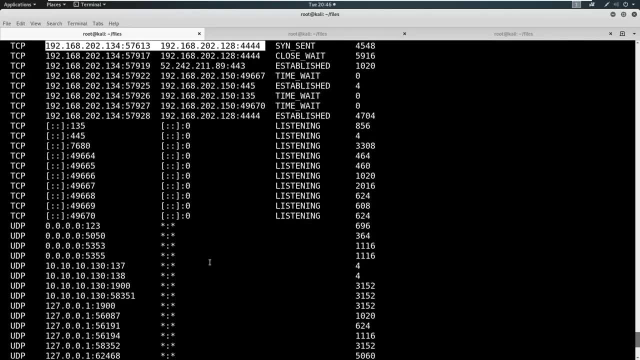 A machine talking to another machine for some purpose or another. So if you see a connection here over one port to another, you might see that. you might see that in the real world as well, But just things to look out for. this is how you'd be able to identify that a machine is dual, homed outside of the IP. 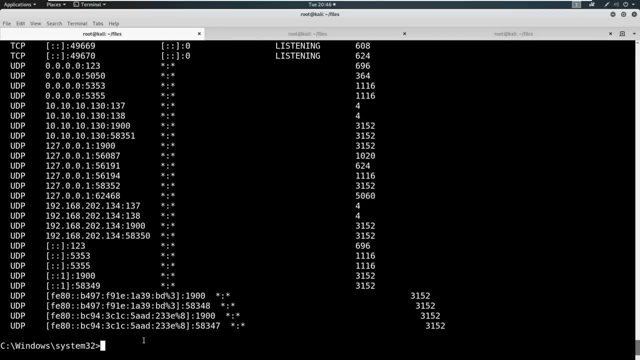 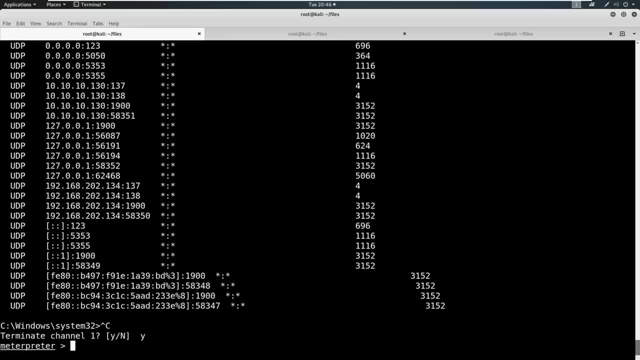 config right and You just want to notice these things. so Control C. Now we've got our auto route going. Now, in theory, we should be able to communicate with that machine that we weren't able to communicate with Wink wink. right, so We can do some things. we could say use auxilary. 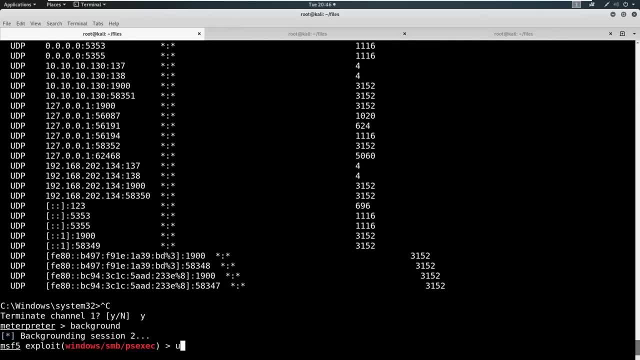 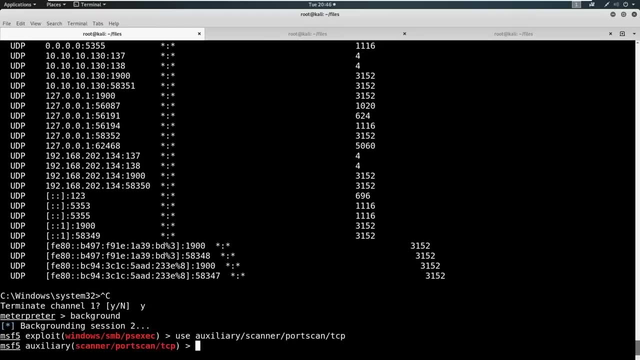 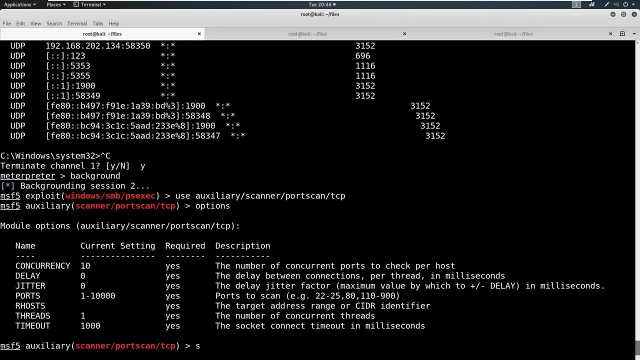 Actually you could bet a background this. We could say: use auxilary scanner, Port scan, and then we could do a TCP scan right, and If we say, options, Okay, so we can set the our host to 10.10.10.1. 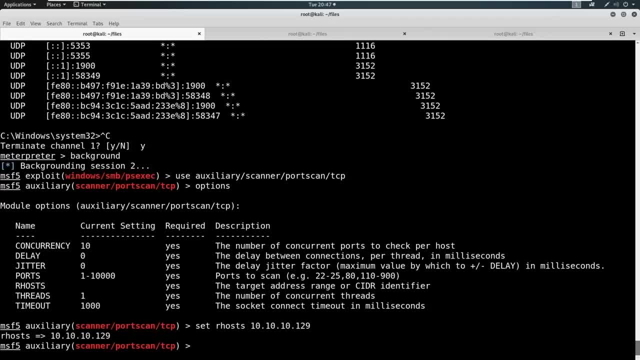 29, and Then we get to set the ports right. It's gonna scan one through 10,000. scanning on a pivot is Incredibly slow. So just for a proof of concept, What I'm going to do is: we're just gonna. we know the SMB is open because we open folders on this in the past. 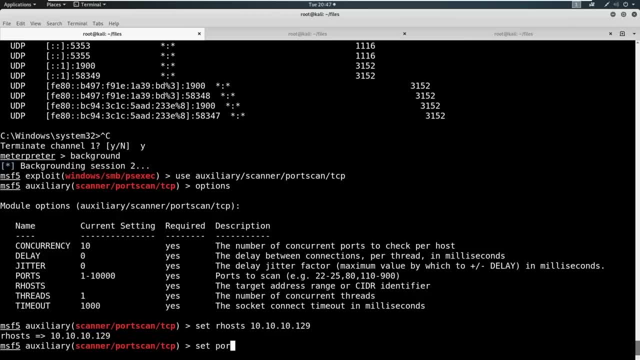 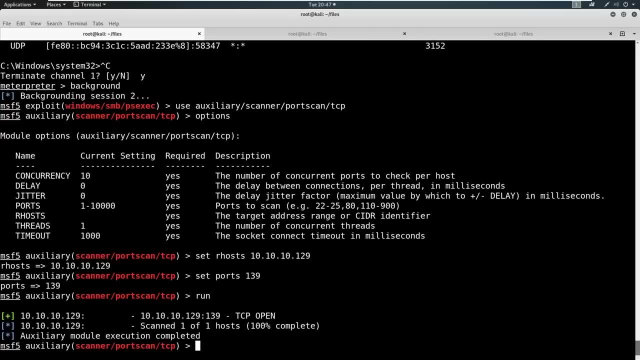 So we're just gonna say: set ports 139 and then we're just gonna run this: Okay, and you see that it says port 139 is open on that machine, right? So we're going through the machine that we exploited and we're scanning against it. 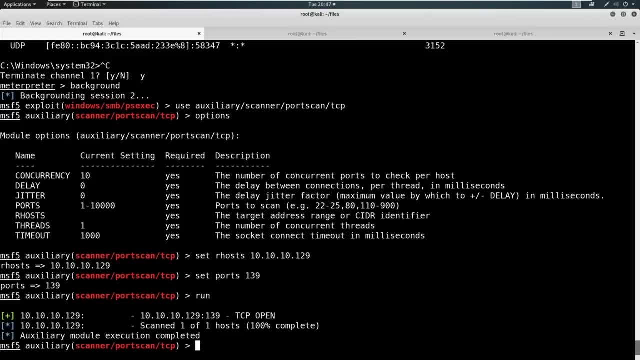 Now, I wasn't able to get this to work, But I will try for some on-screen magic and see if we can get it to work. We could try using The exploit again. say that we dumped hashes or we knew credentials or something right, And we've got local hashes and we want to pass the hash around to this new network. 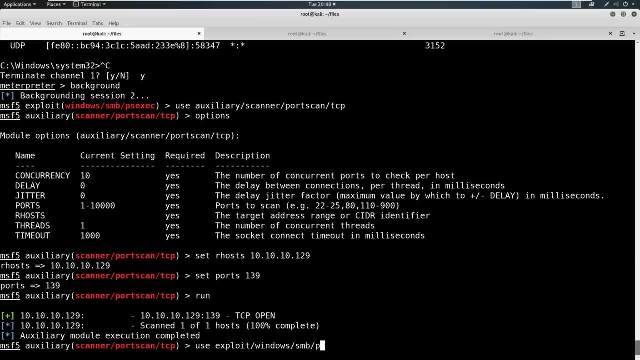 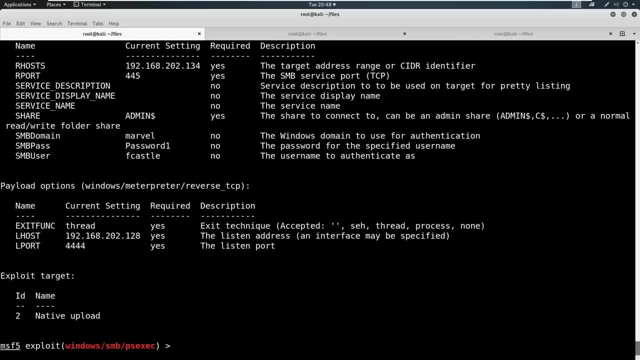 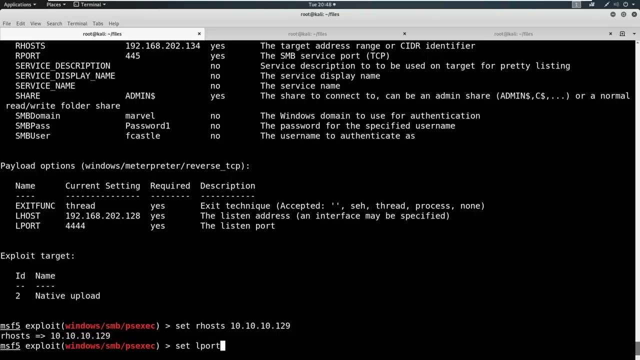 We could try to use the exploit again with SMB PS exec and see if they work. if we go options, we know that the The our host is 10 dot 10, dot, 10, dot 129 And I'm going to change the L port to all fives. 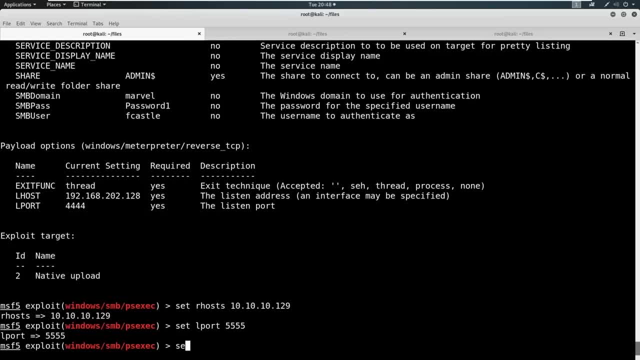 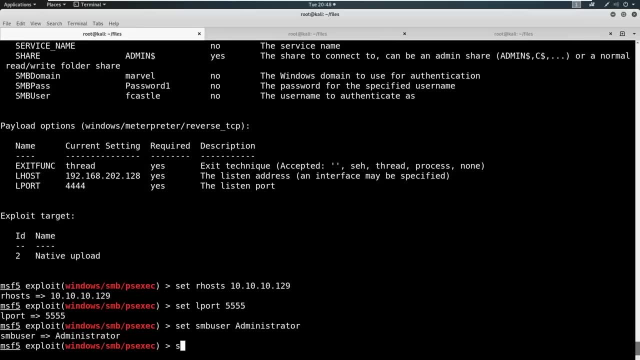 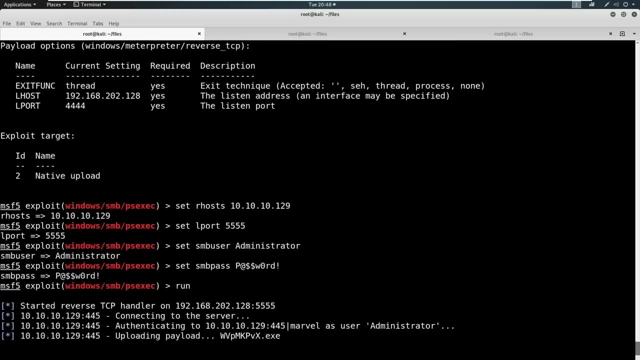 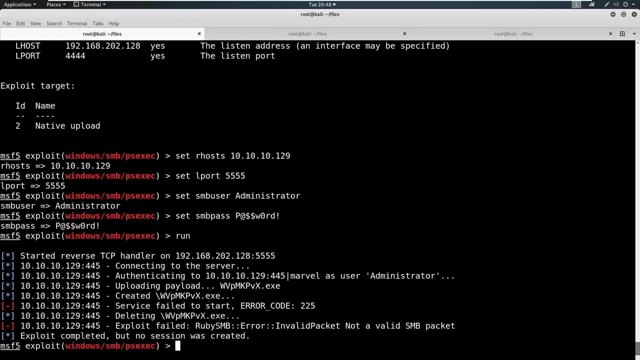 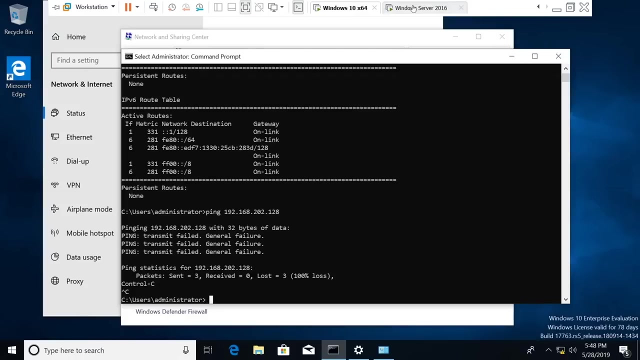 now the Marvel is still the same, but let's change the SMB user to administrator. Just for proof of concept, set the SMB pass to what we've been using. Let's hit run, Let's hit run. I heard a ding in the background. Chances are it blocked. it with defender would be my guess. 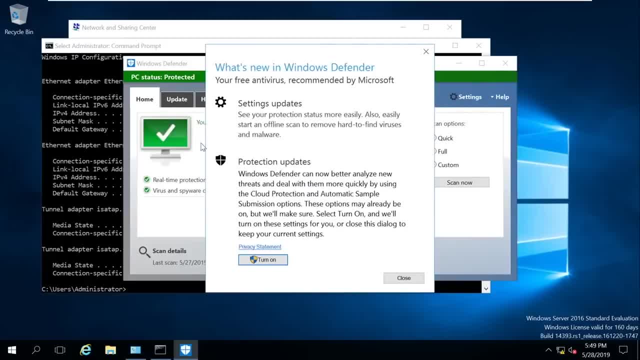 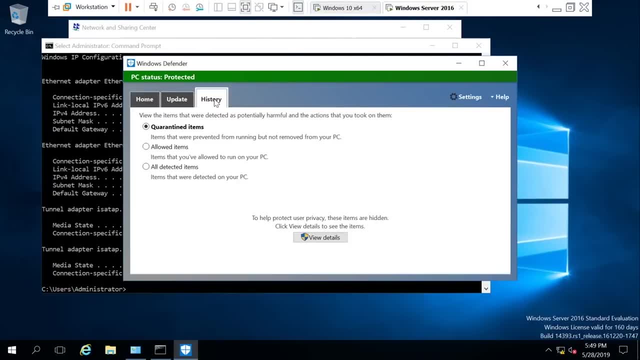 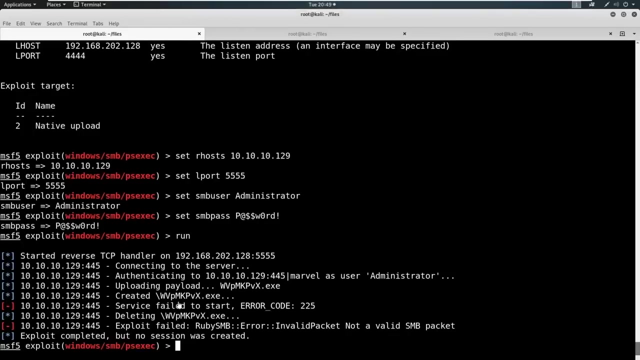 Okay, yeah, I'm not gonna worry too much about it. We can view the details. It sounded like it. it blocked it. that's typically what happens, But just know, as a proof of concept, that you can run these exploits through one machine to another. this is the idea of pivoting. 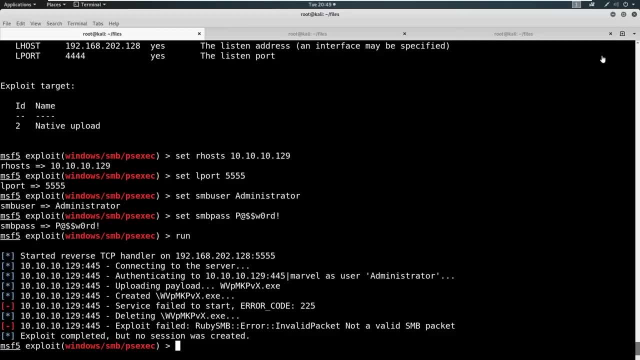 um, I And yeah. So if you see a dual home machine, you might be able to transition off of one network into another network, Leverage that access and navigate around. Would you often exploit users with Windows Defender disabled on pen tests? You would be surprised a lot of places aren't using Windows Defender. 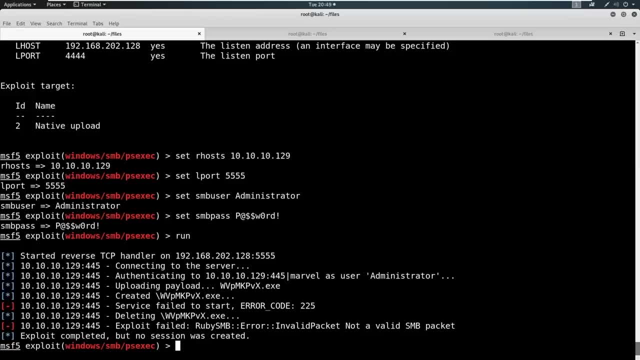 Windows Defender is really just stepped up. its game is what's going on, But it doesn't mean that places are packed And allowing their Windows machines to update for these. They might be using other antivirus that doesn't pick up on this. you might use obfuscated malware. 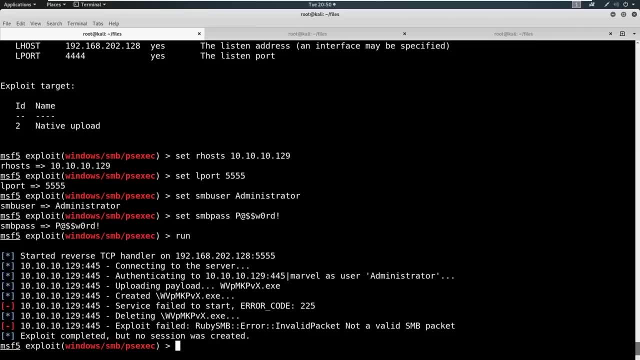 And concepts to try to log in instead. That's why the PS exec has got the PowerShell. It's got, You know, it's got- different options. You might try to to do different things to get around it. So good question though. All right, and that's really it for the pivoting section. let's talk really quick about cleanup. 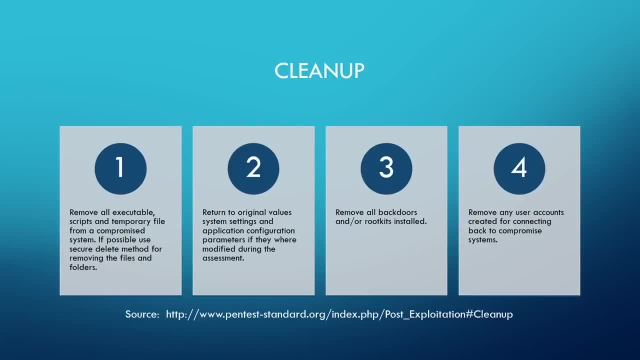 So again, we're going to just talk cleanup, We're not going to actually demonstrate. and now, this cleanup that I'm providing is in regards to pen testing. the other cleanup that you hear about in the hacking methodologies Is more about, you know, removing your tracks completely, you know, like eliminating logs. 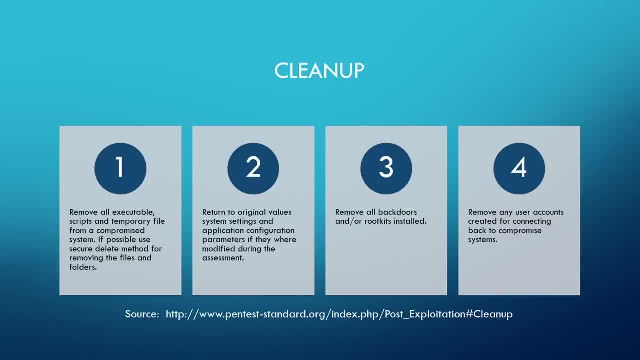 Any sort of system events proof that you were there at all. right, This type of cleanup here is is more geared towards pen testing. This is what this is: an actual- you know realistic- network pen test course. so Just a few notes, and the source is down here, from where I stole all these from. 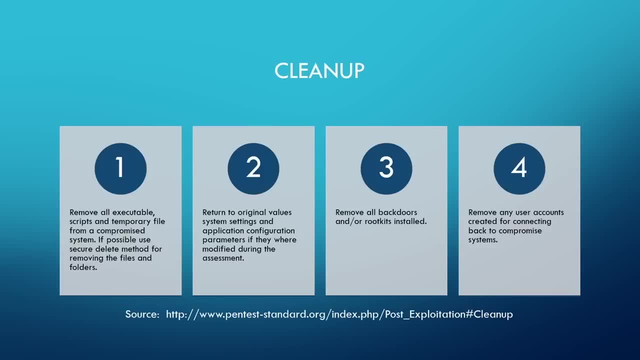 But you're gonna want to remove any executable scripts or temporary files From a compromised system. if possible, use secure delete method for removing the files. right, You want to get rid of all the malware you put on a system. You don't want to leave that. 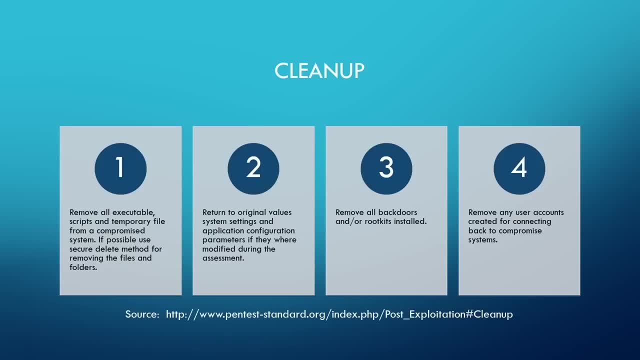 You want to return all the original values for the application parameters if you modified them. You want to remove any backdoors, like you saw with the persistence, any of those, any user accounts You created. a lot of times you'll create an account to access a machine or to plant a flag or whatever. 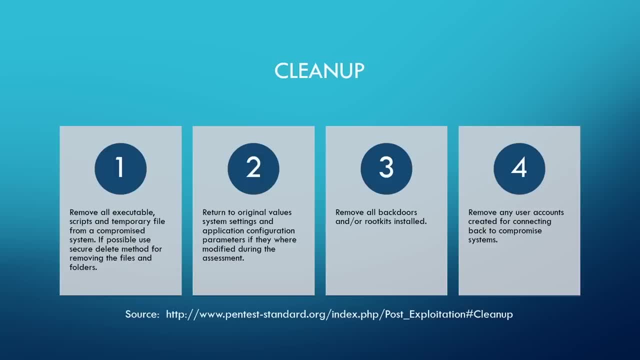 any of these accounts, you want to Delete them. when you're done so, You want to leave it like you found it right. You don't want anything in there that is malicious or could lead to a breach or something, a weakness for the the client At a later time. so you need to make sure that you're you're cleaning up. 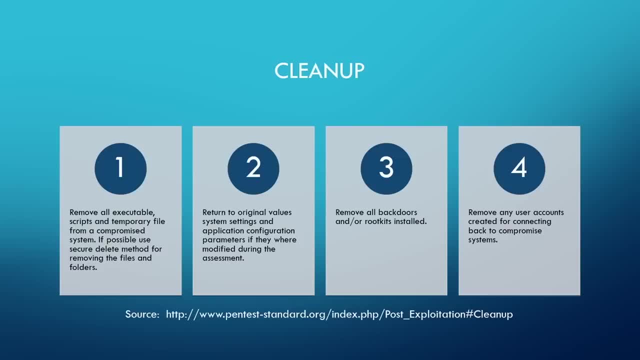 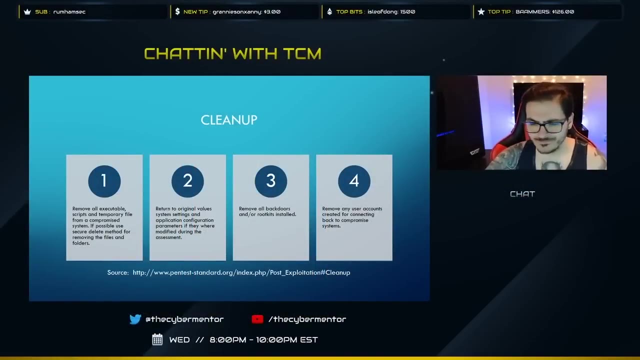 Your mess is essentially the the whole point behind this. So that's, that's all my speech for cleanup, and that's really it. Let me bring you guys back. I'm gonna grab a drink of my monster, And we are on decent timing, actually, Okay, so next slide. 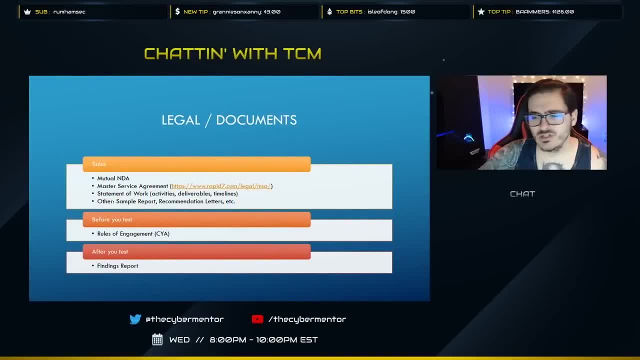 we're gonna get into the legal and the documentation. So we're gonna talk really quick about the sales, Some of the before you test and the after you test. We're gonna go through the, through a sample report and talk about that as well. So in the sales process, when you first meet your client or you sit down, you want to talk to your client and most of these 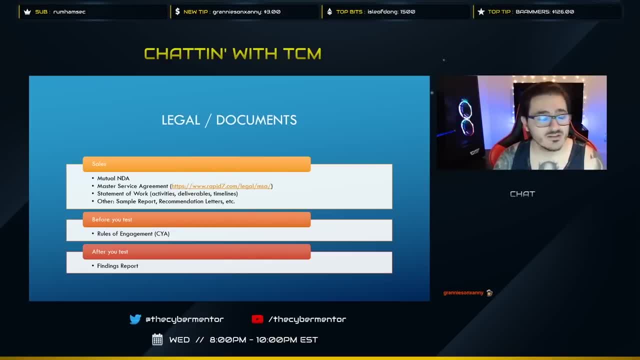 You're probably never gonna deal with. maybe, as a manager level, you might deal with some of these, But you're gonna have a mutual non-disclosure agreement, Meaning that you're not gonna give out the client information and the clients not gonna give out your information that you don't want them to give. 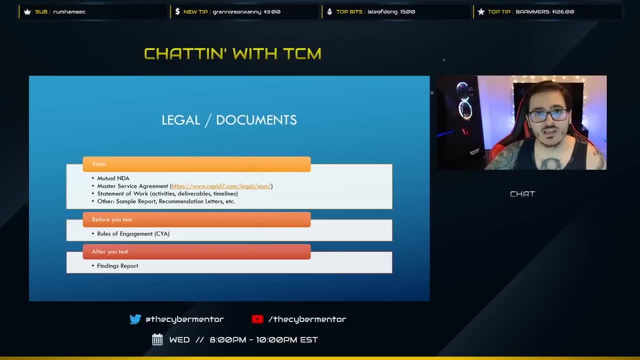 Out. so whether that's pricing structure Or your sales methodology or any documentation You'd give them, it's all under NDA and whatever they tell you about their network, You can't go tell somebody else about that. right On top of that, you're likely to have some sort of master service agreement. 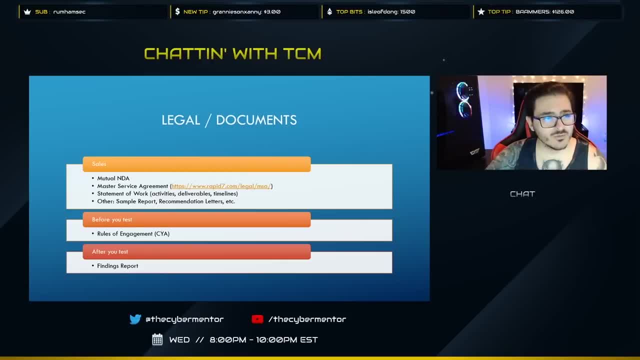 Now I linked one for rapid 7. all you really have to do is just type in Master Service Agreement, pen testing and all of these the big names will come up with their own master service agreement. They're all public knowledge out there. It's basically just a contractual document. um, so it just says like these are the performance objectives and 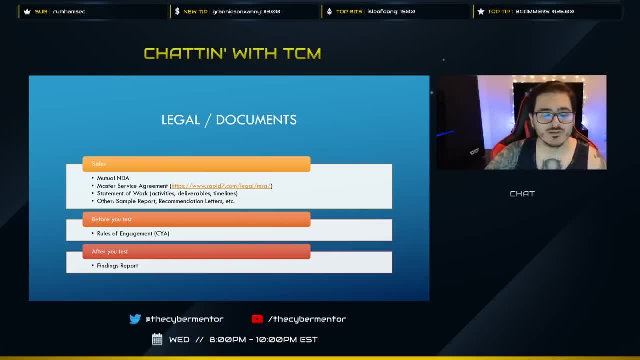 you know what the the responsibilities are, both parties. there's just all legal mumbo jumbo, but it's the, the agreement you sign before doing work. on top of that there is a statement of work, which is your: what activities you're going to do, what deliverables are you going to provide, what? 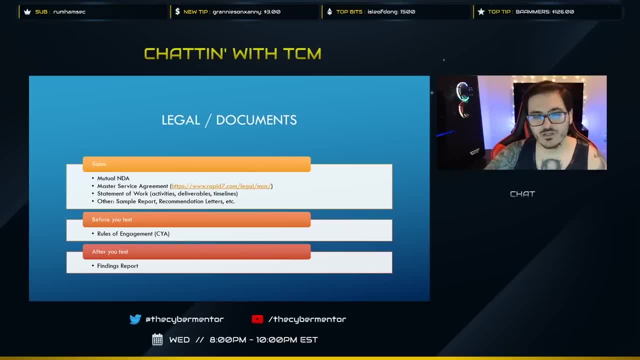 timeline. you're going to provide them on right. um, so, like i'm going to do a web application assessment, i'm going to deliver you a report when it's done and i will get you that in two weeks time and that's your statement of work. um, you're likely going to have costs on there. what the costs? 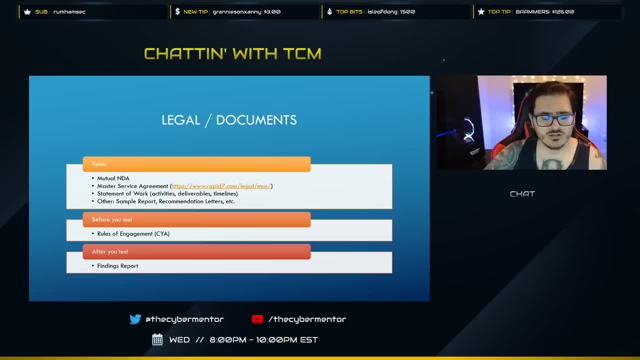 are going to be um and what the um payment terms are going to be as well. so- and sometimes you'll see that the statement of work also, sometimes the rules of engagement as well, um, some places i see split them out, some places they're both the same thing. once the statement of work is signed, this rules of engagement signed. 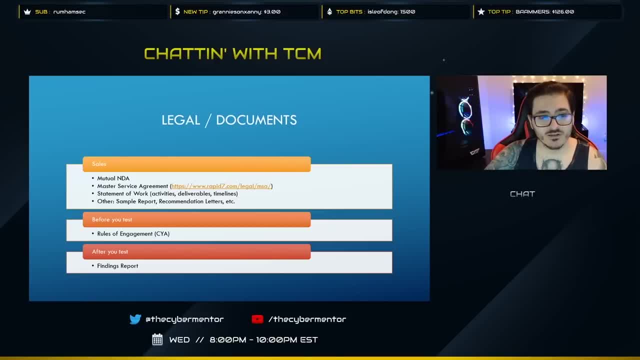 um. so but before you test regardless, you need that statement of work slash rules of engagement to um to go right, because your rules of engagement also has your scope details, like you can't attack this specific machine, or you can't use social engineering, or you can't perform. 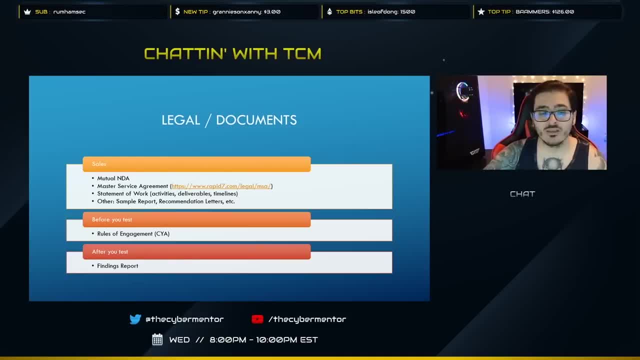 denial of service or you can't use a certain tool, right like, you need to know what you can and can't do, what machines you can and can't attack. um, that's very critical that you stay in scope, because if you go out of scope you can get in. 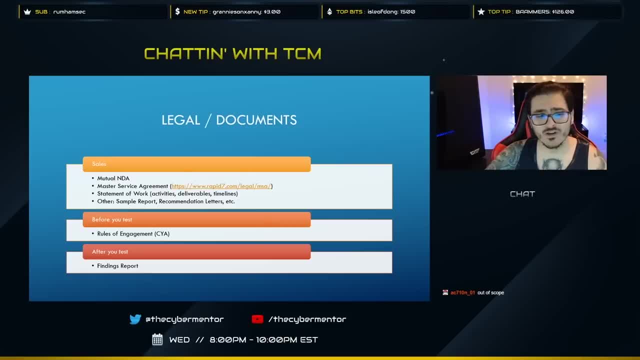 pretty big trouble. so i said, cya, cover your ass. this is a cover your ass document. right? other process: in the sales you're going to probably have a sample report that you give to the client. you probably want to have recommendation letters etc. so any of these things that you can. 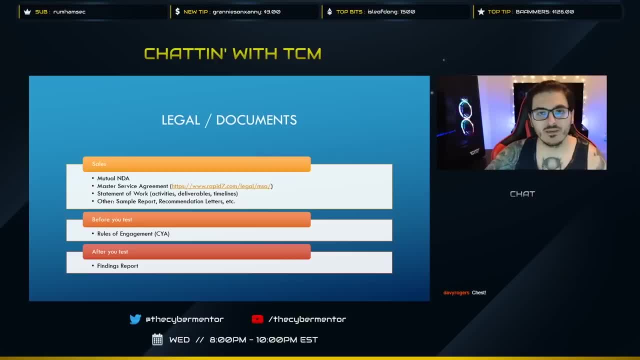 give to a client or potential client. you're going to have a sample report that you give to the client and say: hey, here's more about me, the process, whatever. um, this all helps in the sales side of thing. um. so, after you are all said and done, you do your testing, you have a report to deliver. 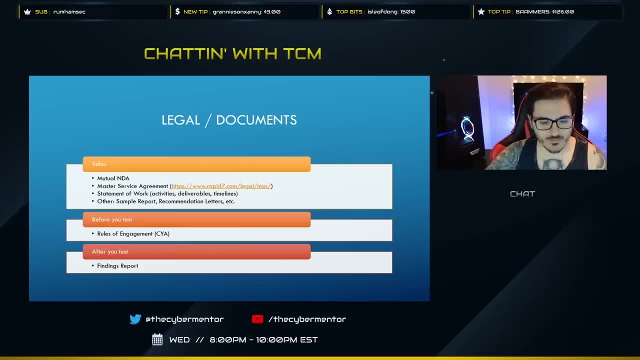 now. i have released this report on github, um, i'm also going to show it to you here. there's a video on youtube, it's all over the place. so if you want to see this again and you don't like this presentation, then you can go watch it elsewhere, download it, play with it, do whatever. so if you, 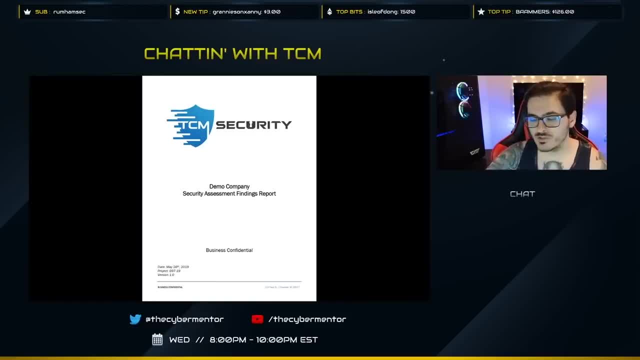 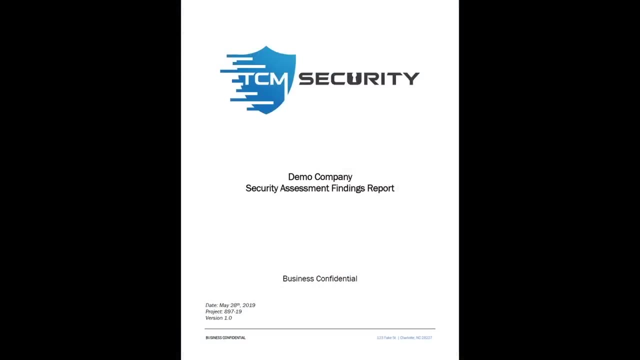 so this is your, yours to use, yours, to modify, yours, to do with whatever you want. um, just, uh, make it your own, you know. so, um, this is just a standard idea. i'm actually going to make this a full screen, so standard idea of how i would organize this um, when i actually give this to clients, i'm going to 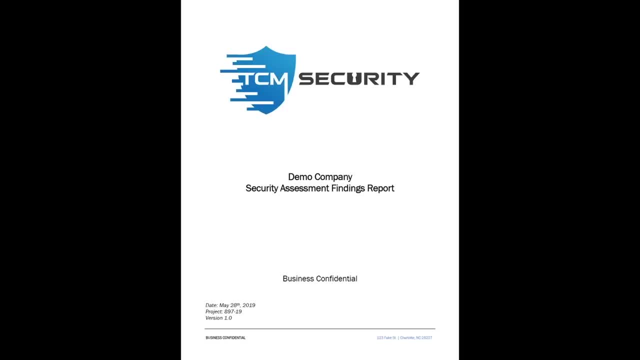 have a little bit more details in here, so this is going to be bare bones for you guys. um, but it's pretty same or close structure when i actually give this to clients as a sample report. uh, so you see, here i've got the header. it says: demo company security assessment findings report. 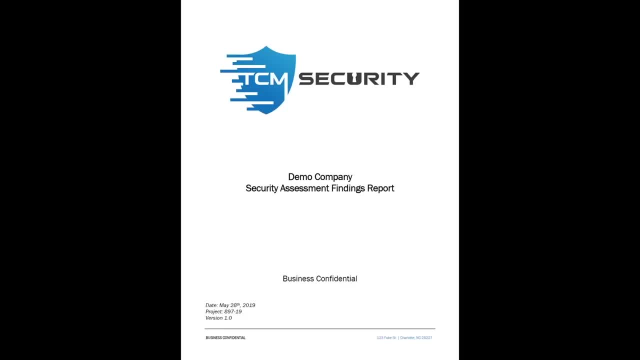 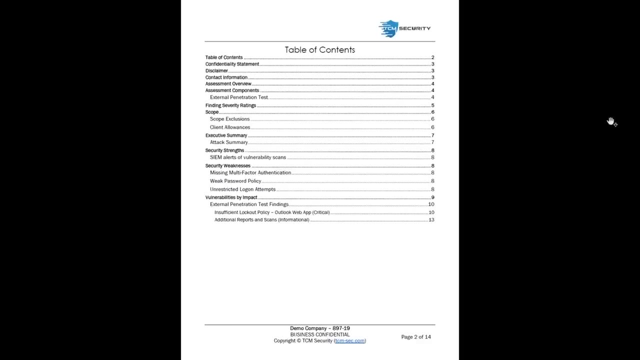 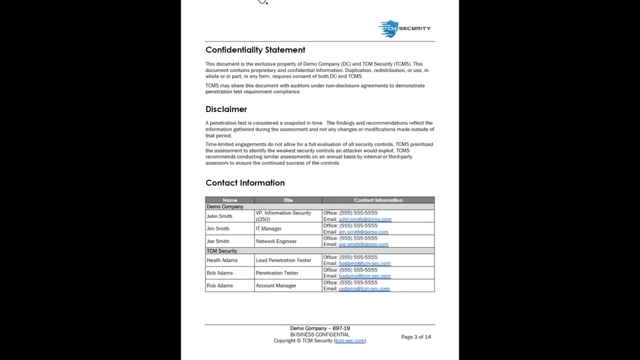 it's business confidential. uh, it's got today's date on it. it's got a project number, version number- again, business confidential. blah, blah, blah. you've got a fancy table of contents, okay, and then at the top you've got a confidentiality statement. it just says that this is between demo company and tcm security and it contains confidential. 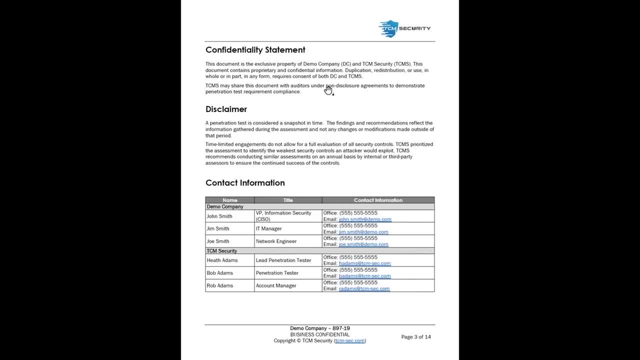 information. uh, basically, you're not going to duplicate, redistribute this in any part and form without the consent of both parties. um, so, on top of that, it says you can share this document. um, if we need to, actually this says tcms. this should probably say dc. you can share this document with. 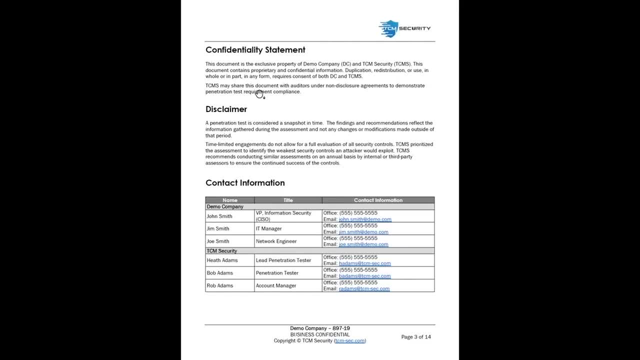 auditors under non-disclosure agreement and you can share this document with auditors under non-disclosure agreement to demonstrate penetration test requirement compliance. um, so sometimes you have audits and compliance requirements, so it's not saying that you can't share it, but as long as the other people. 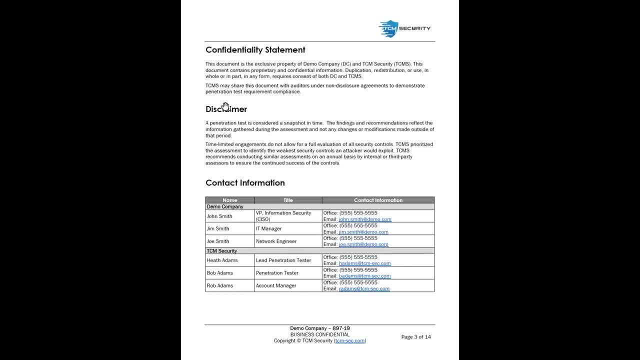 are under non-disclosure, that's fine. um, here is a disclaimer. the big thing that you want to note to potential or to clients is that a penetration test is considered a snapshot in time. the day after you finish your test, an exploit can come out, a misconfiguration can occur, something. 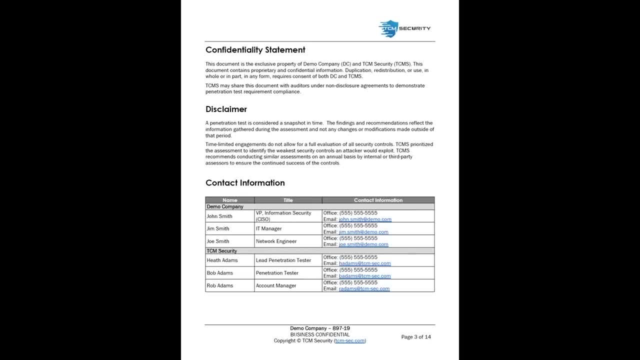 that causes a vulnerability right and you want to make sure that they're aware of that. you also want to make sure that they're aware that this was a time limited engagement. if you're only given a week, chances are you're not going to find every single thing on an assessment, especially if the 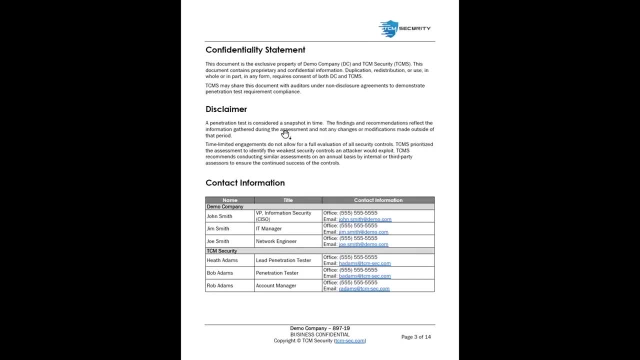 assessment's full of vulnerabilities. so what we say is: we prioritize them to point out the weakest controls, and then we gave them full report information for further details. um, on top of that, you always want to include contact information. so who are the important contacts from the company you're pen testing? who are your important contacts here? 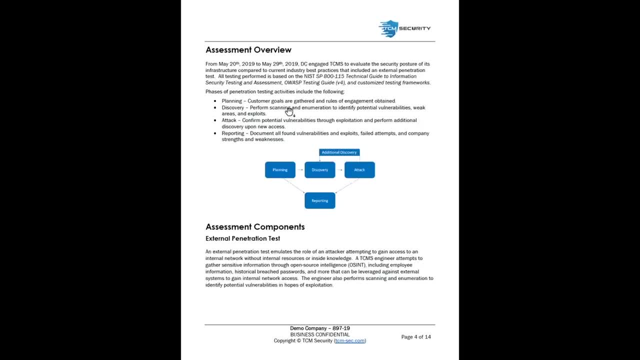 okay, you're going to give an assessment overview. you're going to say, hey, we were engaged from these dates to these dates and we evaluated the security posture based on best practice, and that included. this is just an external penetration test for this one, but if you had more components and you 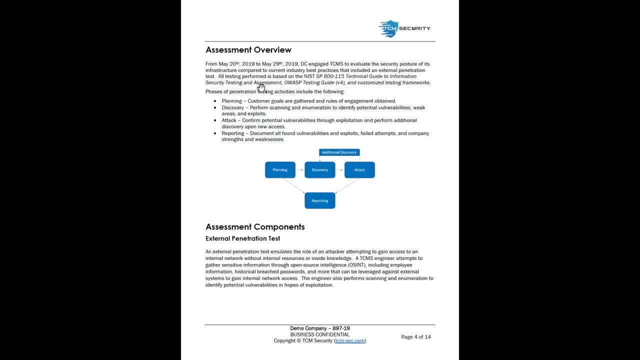 would list those in there. you would say, hey, we're engaged from these dates to these dates and we would list those in there. um, all testing is performed on the nist sp800 guideline. also, we do tests on the olaf's testing guideline and customized testing frameworks. 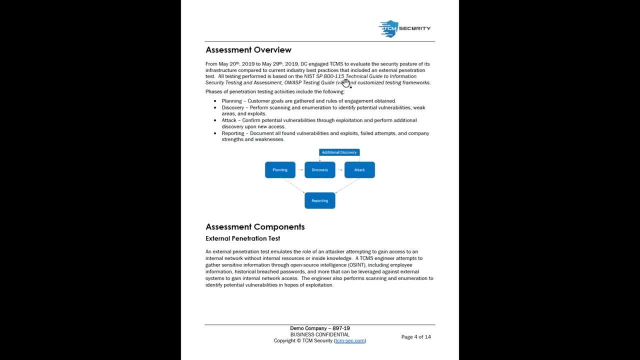 these phases of a penetration test come from the nist sp800. so there's planning, discovery, attack, reporting. you just talk about what that is. i made a tiny little infographic here that shows you know you do planning, you do discovery, you do attack, you report on what you attack. but then, if you also get, 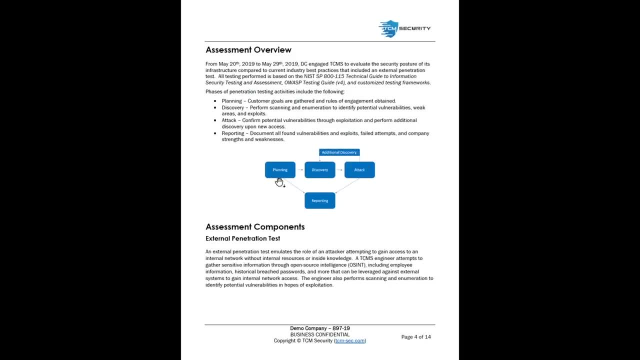 in. you do some additional discovery, repeat the same process and you're good to go. so that's what we're going to be doing in the process and report. um so, with that, you also want to include the assessment components that you perform, right? so you're performing an external penetration test, so this: 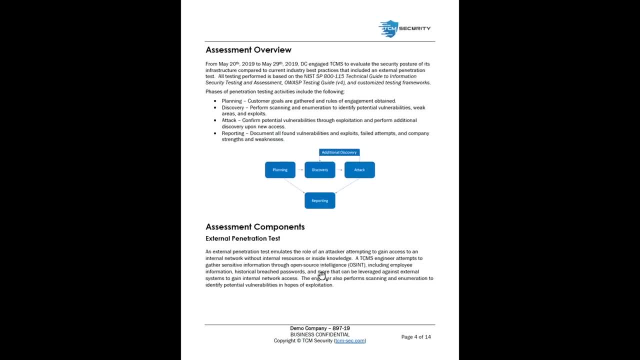 just gives you a high level overview of what a external penetration test is. it says we're going to use osint employee information, historical breach information, we're going to perform scanning enumeration to identify potential vulnerability in hopes of exploitation. so if you had an internal, you would note what that is. you would note web app, you know social engineering, whatever the. 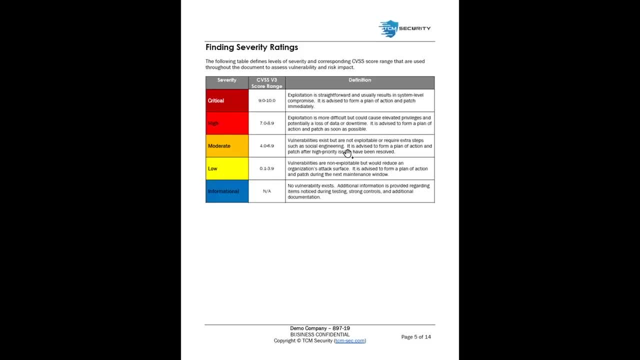 engagement, you would have a list of all your components. so coming through here now we've got a finding severity rating. this just says what the ratings might be, from critical to informational, what the cvss v3 score is- uh, comparatively for those- and what the definition is like a critical. 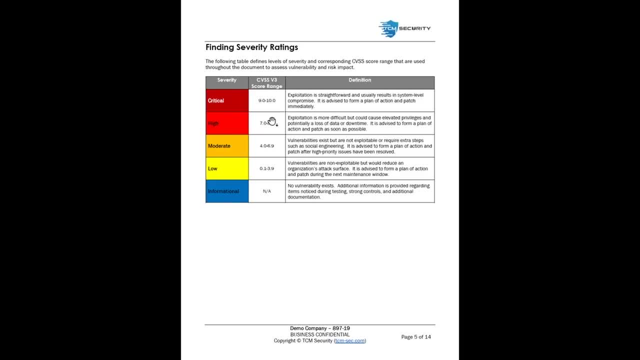 is exploitation super easy. um, it led to like a system level compromise, an rce some sort. you need to plan an action right now and patch immediately where a low is like, yeah, it doesn't lead to an exploit, but you know, best practice states that you should probably patch it. 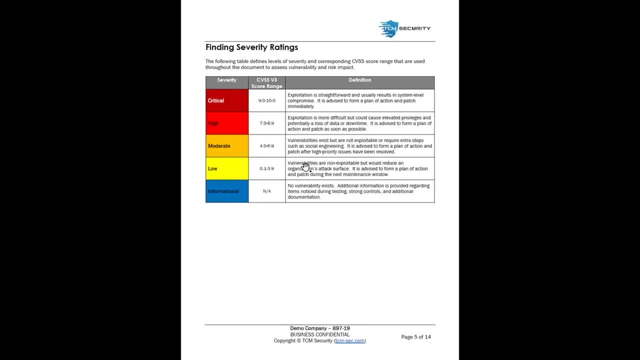 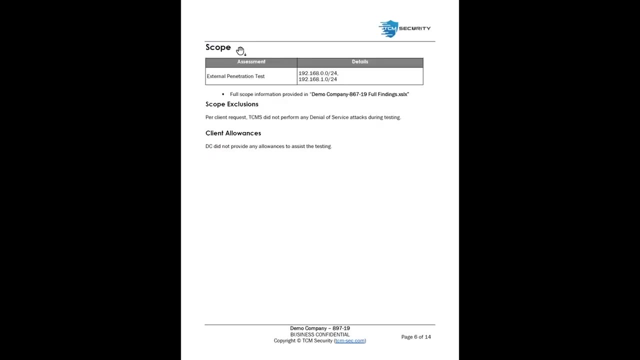 in the next maintenance window. um, but you know not a big deal if you don't. so, um, we have this findings chart, just so you know the customer is aware what, um, what each finding means. and then, going through that, this page is a little lackluster. I want to add some more to this, But you always want to include the scope. 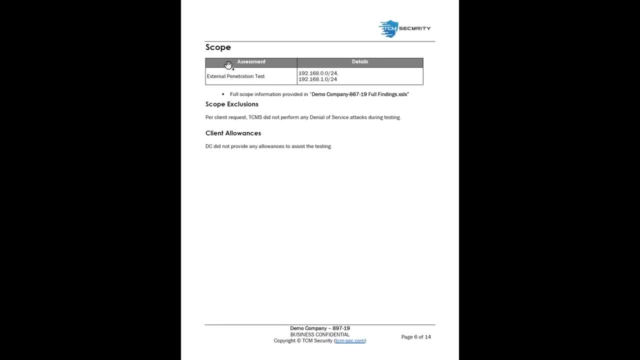 And there would be a. you know there'd be more information here for every assessment component. you did So if there was an external and internal web app, you would give all the details of what you tested. Now I know these are internal IP addresses. I'm wasn't going to put external IP. 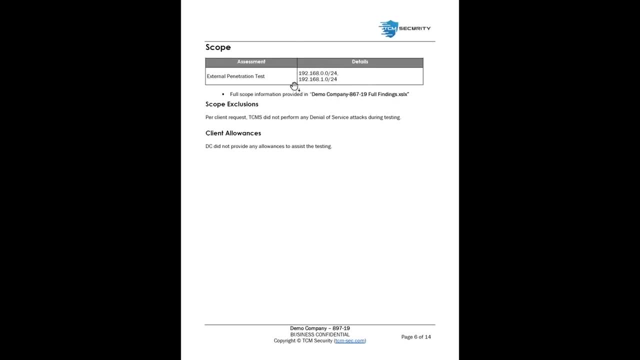 addresses out there, because somebody probably owns those. But you would just say, hey, I tested this range and this range whatever. And then full scope information is provided in a additional full findings Excel document. That's where you list out all the findings that you found with. 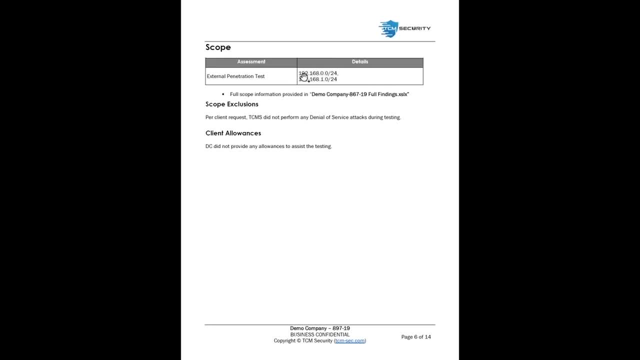 notes on them. And then you would say, like if you had 50 IPs you were testing against. you might not list them all here. you might just say I'm testing against 50 IP addresses. Other than that, you want to have the scope exclusions, right, So we didn't perform any. 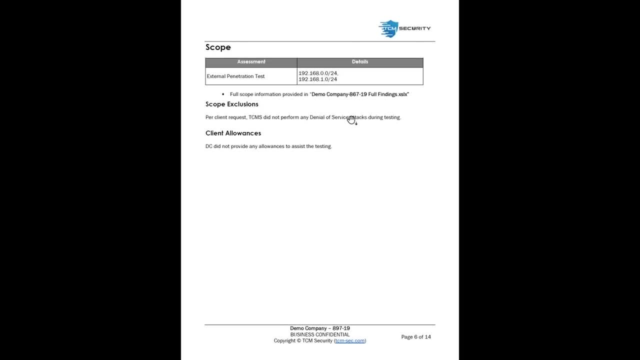 denial of service attacks during testing. On top of that, we have client allowances, right, So did they provide us a password? Did they provide us, you know, any sort of things that allowed us any kind of help on this testing? you want to notate that. So, on top of that, scroll down. 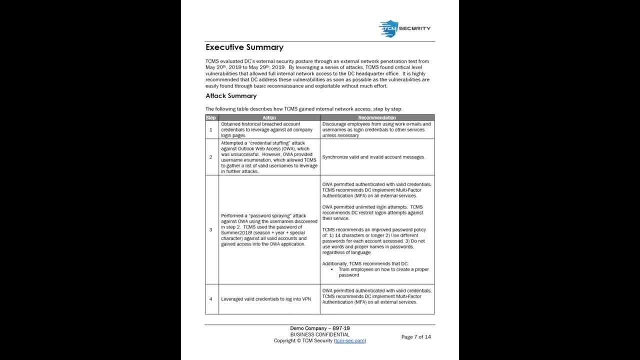 Now you want to do an executive summary and you want to do a technical summary, right, So the executive summary is for your C level. the C level just likes to see things. they like to see pretty pictures. they don't really care about the muddy details, right, So you want to give them. 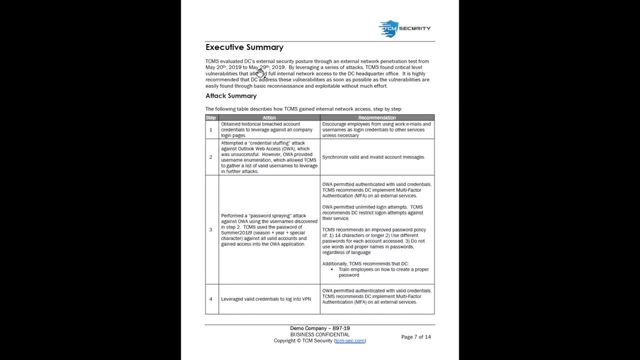 everything up front that you can give them. So a quick blurb here. it says we did the testing from this date to this date By leveraging a series of attacks. we found critical vulnerabilities and we were able to gain full internal network access to the headquarter office. 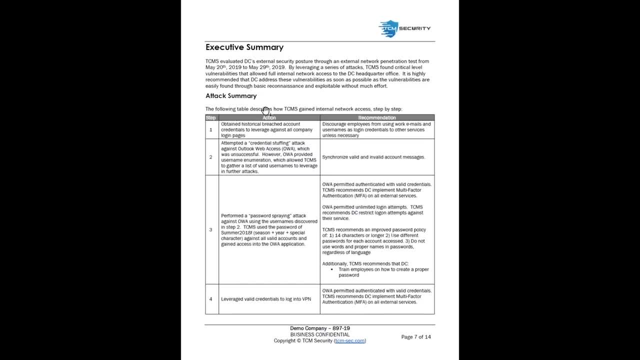 Um, and then we gave an attack summary of how we were able to gain internal internal access and some of the recommended remediations. So from here, like we obtained historical breach account credentials to leverage against the company login pages, So a recommendation there is to discourage your employees from using work emails and usernames as login credentials. 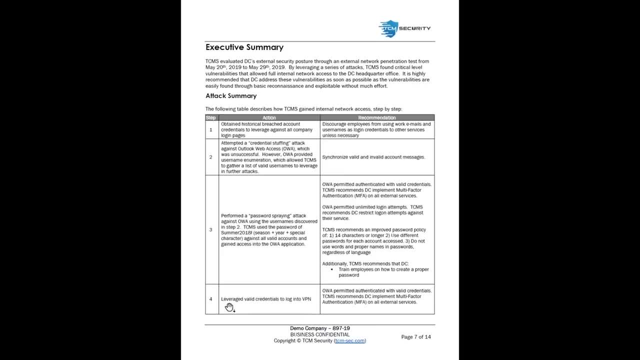 to other services unless necessary. All the way down to, we leveraged valid credentials to log into the VPN. Well, they permitted VPN access, right? Yes, they did, They did, And the VPN did without multi factor authentication. So we recommend that. 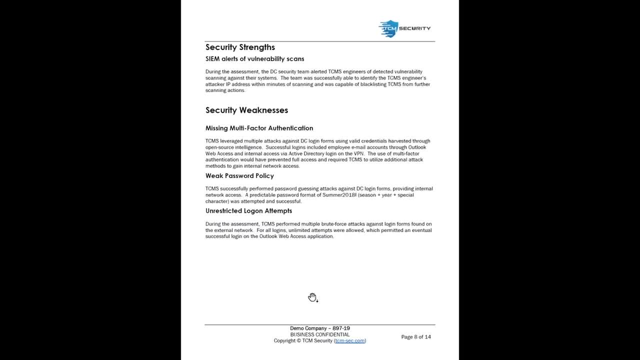 they use authentication on all services, So on all external phasing services. So here you would provide some strengths and weaknesses. So an example of a strength is okay. well, their sim was alerting on vulnerability scans. as soon as we started scanning, they alerted us that they saw us. 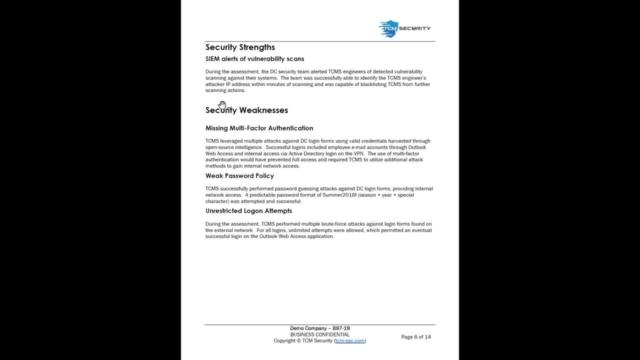 they verified our IP address and they have the opportunity to blacklist us from further action. you would probably want to provide here at least three to five good strengths that they had And you would want to provide, you know, if they had- weaknesses- three to five weaknesses and probably fill out two pages of 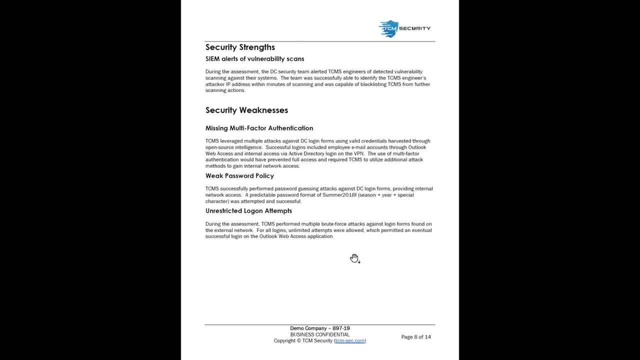 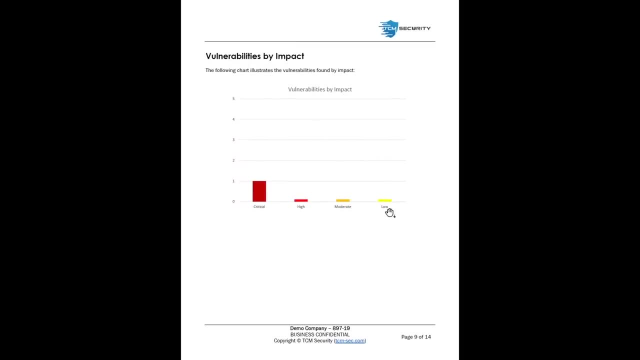 this. So the more information that you can provide, the better. Again, this is just a bare bones report, So here is a. vulnerabilities by impact. Basically, this is a chart that says critical, high, low, moderate, whatever. how many vulnerabilities do we find by each impact? 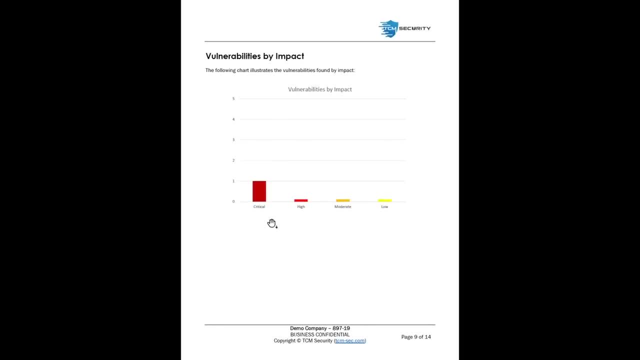 There's only one finding on this report And it was a critical finding. So there's only one critical. you probably put a little bit of blurb down here about why the findings critical or what whatever you know you could add and make this your own. 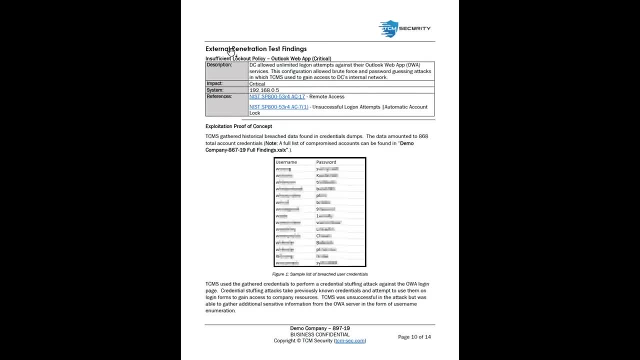 So, on top of that, you come down here now and you have the external penetration test findings, Right, so you've got the insufficient lockout policy. So what it says is: the company allowed us unlimited login attempts against their outlook Web app services. This configuration allow brute force and password guessing attacks in which we were able to gain access to their internal network. The impact is critical because we did gain access. we note the system that we gained access on, and then we provide the references of the pages for this. So, obviously, remote access and then unsuccessful login attempts, automatic account login attempts and actually에서도 login attempts- Such a great tool. Inwardly enough, they were able to attain access to. 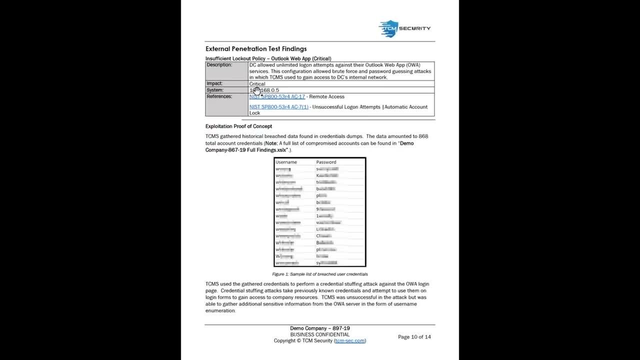 the descon Kardashian and who grateful to Utd's side that helped us get an order back in doors. When we confidentially jump to the support hub, we didn't enjoy us being snubbed and out of line. in this case we did. we thought that through the 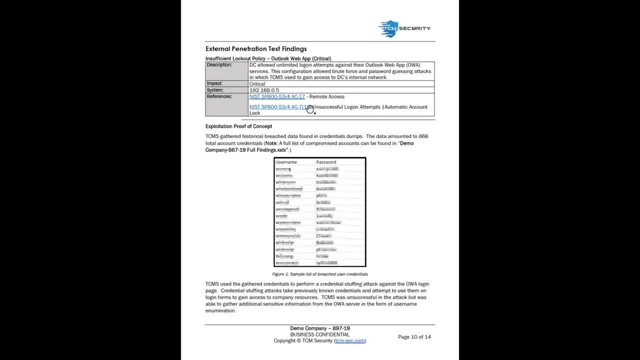 pages for this. So obviously remote access and then unsuccessful login attempts, automatic account lockout, both NIST, SP 800 policies, And then you provide a proof of concept. So first things first, we gather historical breach data found in credential dumps. 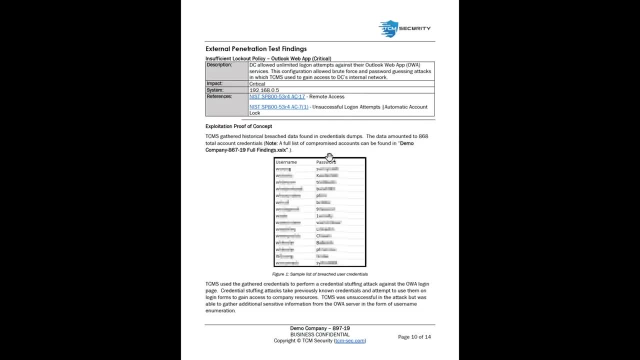 The data amounted to 868 total account credentials. Now, obviously we can't put all those on one page- It would take up many pages. So we're just going to say, hey, we'll throw them in the full findings. That way you can review all the account credentials. Here you've got the usernames and 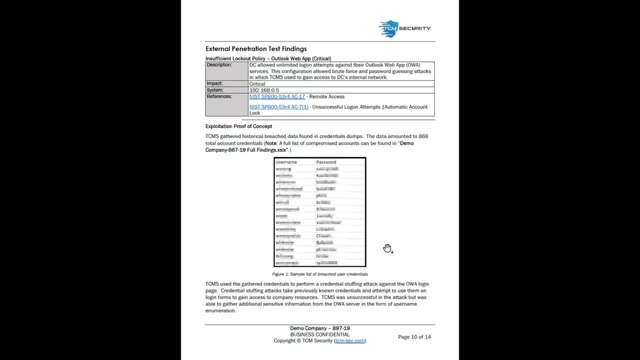 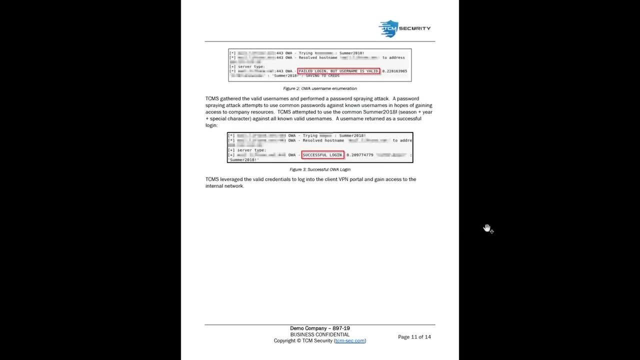 passwords. And then it just says sample list of breach user credentials. And then we're just going to go through the whole process. We took those credentials, performed a credential stuffing attack, blah, blah blah. We weren't able to gain access with credential stuffing, but Outlook was. 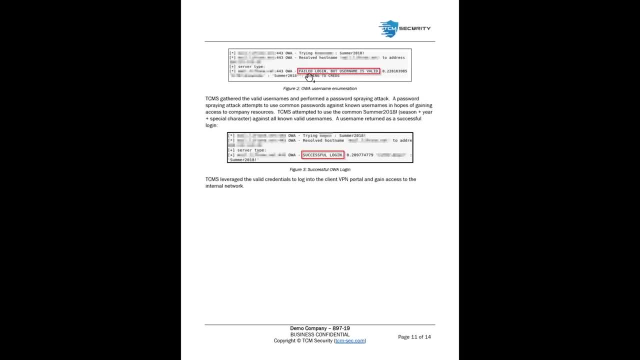 providing enumeration through username enumeration. So got failed login but username is valid, So you using that. we gathered valid usernames and performed a password spraying attack. We use summer 2018, exclamation point: a username. return a successful- you see successful login here. 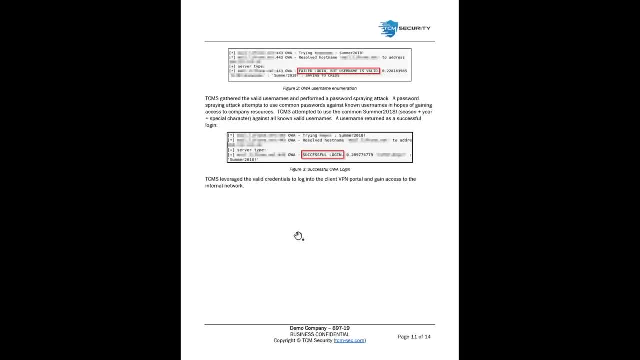 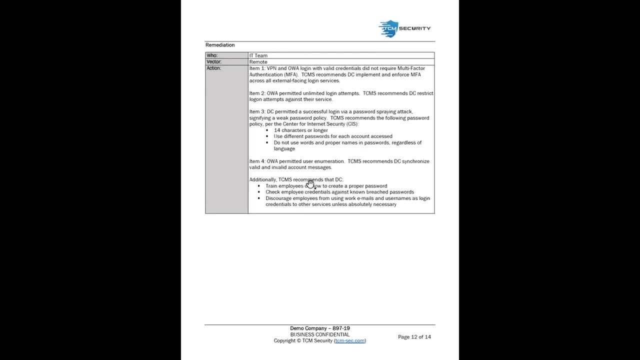 And then we would say we leveraged the valid credentials to gain access to the VPN. there would be a picture here: VPN access From there. you would want to make a remediation recommendation. So I like to put who what the vector is and then what the action is going to. 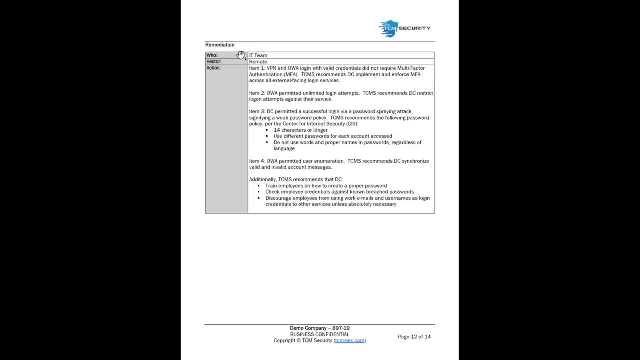 be. So who's going to be the IT team? If this was a web app, you would say developer. or if this was Maybe more workshops side, you would say network engineer. And then you'd say: you know, the 여기에 was done remotely, So it's a remote vector. And then you want to talk. 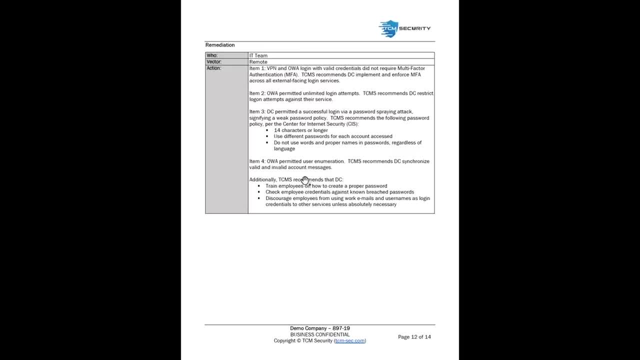 about all of the actions that they need to take just through these steps. So item one was: you know, VPN and Outlook web access or did not log invalid credentials, did not require online access. multi-factor authentication: we recommend that they implement multi-factor, so this: 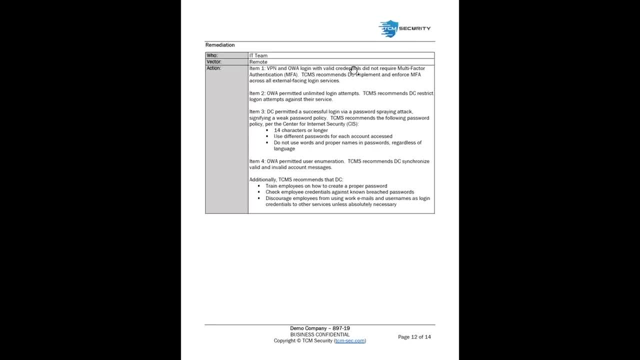 is again the same kind of recommendations you saw at the high level earlier, but you're seeing it down in the weeds again. this gives a little bit more detail, you know. use 14 character passwords or longer. use different passwords for each account access. don't use words or proper names like summer. 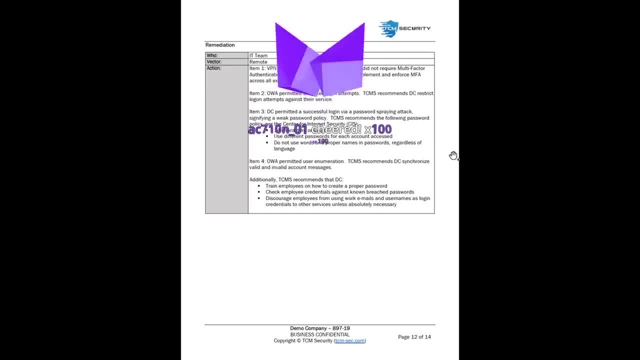 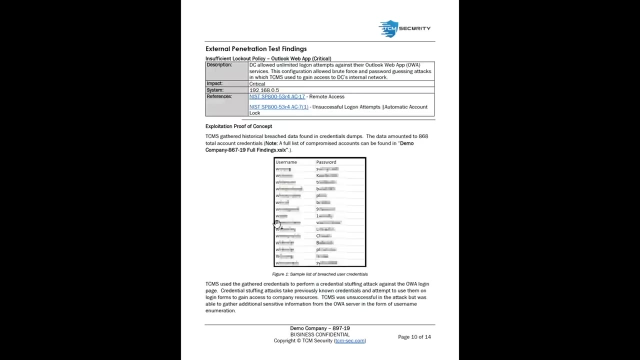 2018. you know, in passwords, thank you, action, appreciate it. and then you, you know, you just come through here and you make all your recommendations, and then you would just continue on with this. you would say, you know, and they might not all be this long and proof-of-concept. this is a long proof-of-concept because 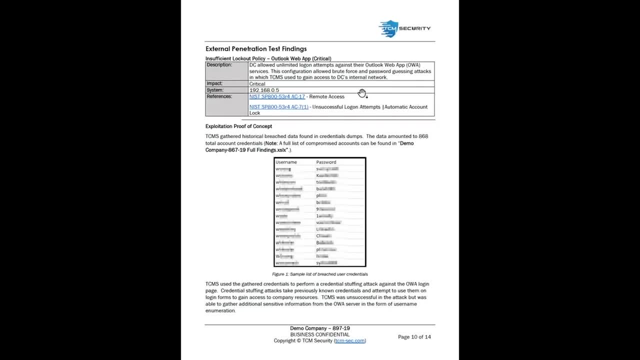 it led to something you might just say: hey, this is out of date, this is a medium finding or a low finding. here's a picture of the version, or proof of a version. right, and you'd say: blah, blah was out of date. here's proof of concept with a picture. 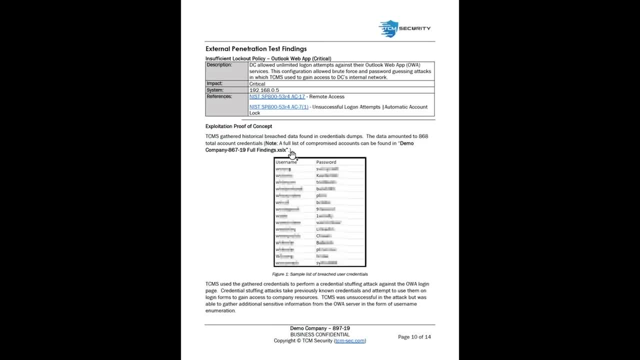 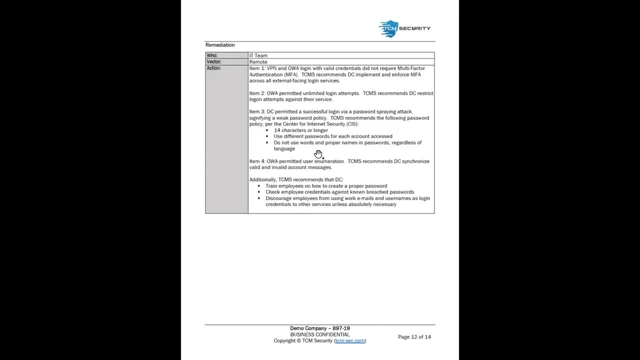 and it might just be easy. and then the remediation might, it might all fit on. a one page says: remediation, you know, update to latest version, blah, blah, blah, and then you put that in the reference. so they're not going to all be long like this, but this is just a good one to show step-by-step and how it works. 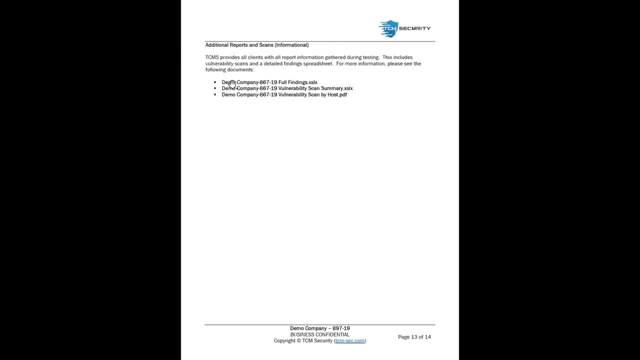 so on the next page there is additional reports and scans. we always give out reports and scans. we always give out not only that full findings report, but you would want to give out all the Nessus documentation, because you don't always get to the the every single. 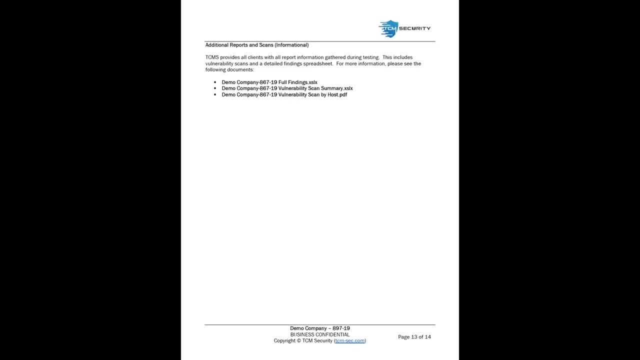 finding right. there might show up a hundred and something items on a Nessus scan and you may only be able to do 20 or 30 to check those in a time-limited test, right, depending on how vulnerable they are and where you spend your time. 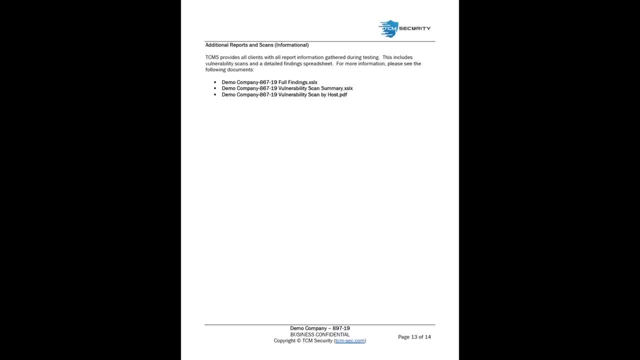 you might not get to everything, so you want to provide all your final findings, the details that you can, to the client so they can go through and review those on their own time. and then, other than that, you have- um, you're just the last page here. uh, some companies will include. 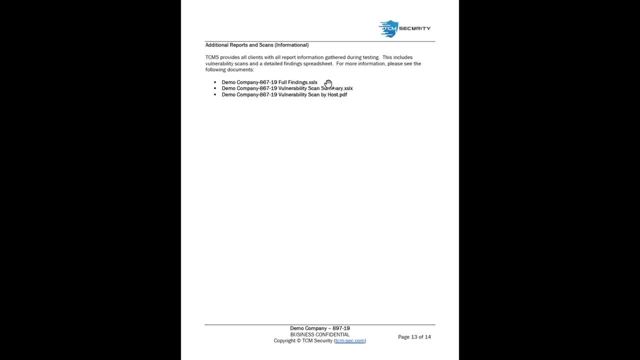 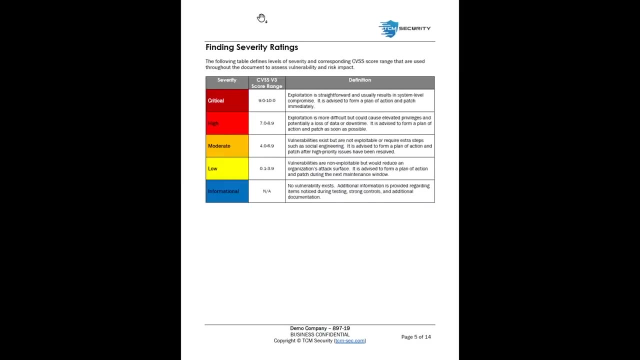 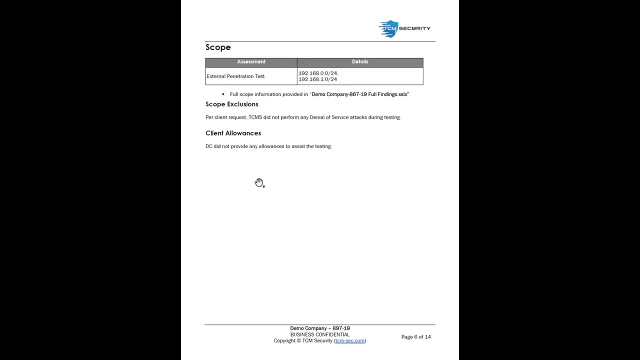 appendices, appendices, um. you you could have whatever you want in there. uh, you could put the methodology that you see down here and there. you could put the um, like the severity ratings down dependency. there might be more detailed information about the scope or or network penetration test, scope or whatever, down in the um in there as well. so, uh, it's up to your. 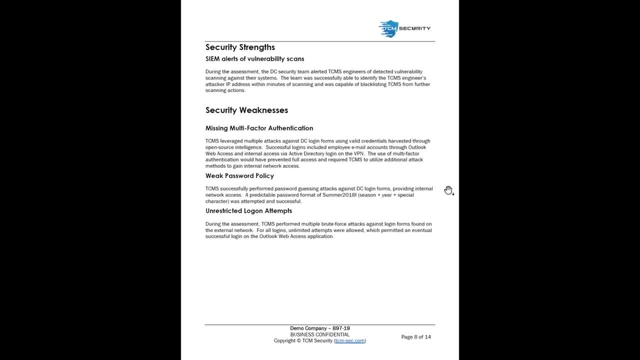 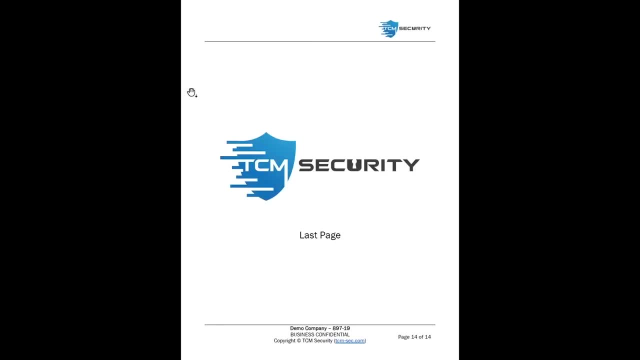 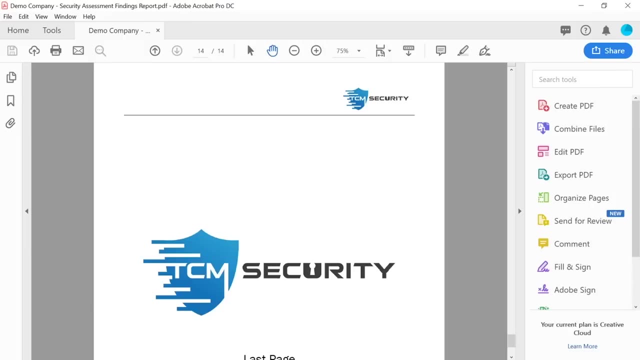 interpretation. so, um, always worth considering other than that. that is it for the reporting side of things. okay, one more slide, i think, and then we should be good to go. and i'm looking at my phone: is buzzing like crazy. it looks like my- uh, my- flight got canceled, so that feels sad. 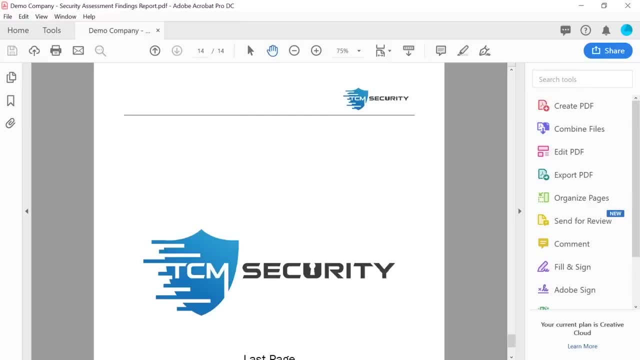 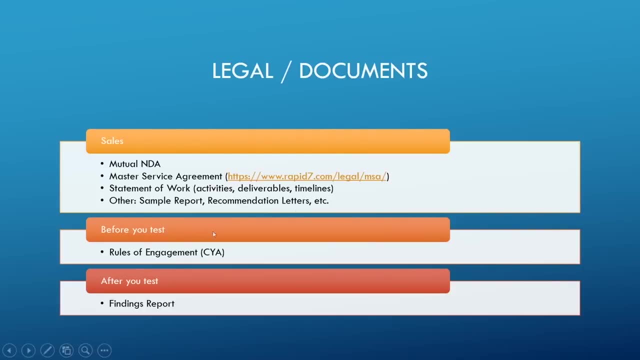 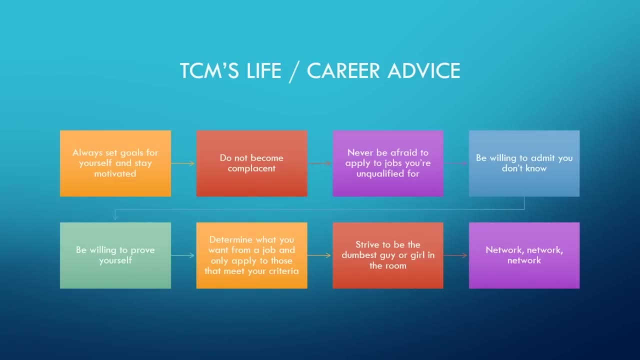 super sad guys, okay? um, so let's open up this and i'm gonna take a drink and then i'm gonna give you my career advice. dude southwest, you're damn right about it. all right, so we're going to talk about these in, uh, i guess in this order that i put here, um. 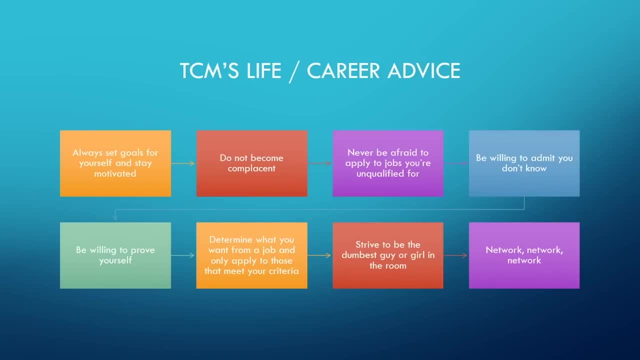 so here is my career advice for those of you seeking to get into the field or work in any field. honestly, uh, career advice number one is always: set goals for yourself and stay motivated. so, um, for me, what i like to do is, if i've got a, 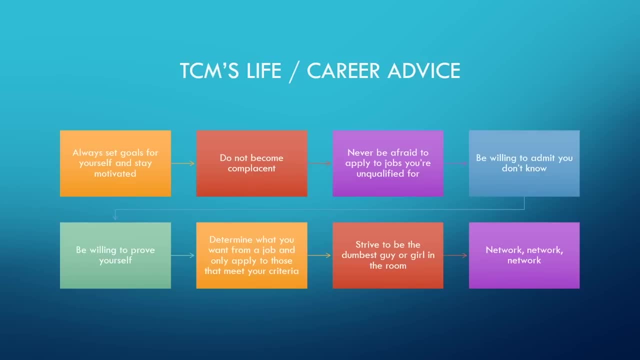 certification or something that i want to get done. i will set that certification up, i'll register for the voucher and i will- um, i will do it, say like i want to get it done a month from now and then i'm going to do it a month from today. i will buy the voucher and register that exam to sit for it in a 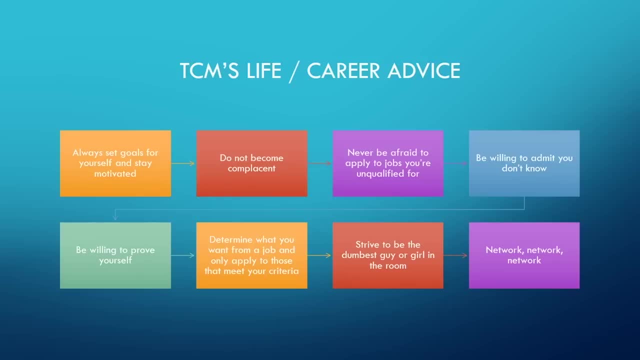 month. um, that way i've got that time pressure right, that goal is already there and that helps keep me motivated. so you kind of want to have these goals and keep motivated- and you've heard me preach about this before. but working in information security, especially the higher up- 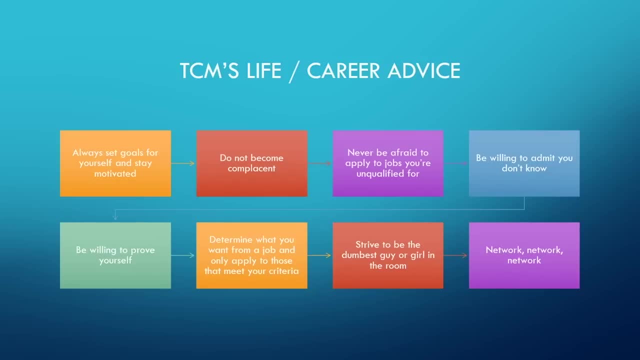 the food chain you get, you're gonna um, you're gonna get left behind if you are not staying motivated, and that falls into as well. it falls into the. do not become complacent. so what that means is- and i'm going to describe my, my journey upcoming right like so: when i first started out, i started out in help desk. 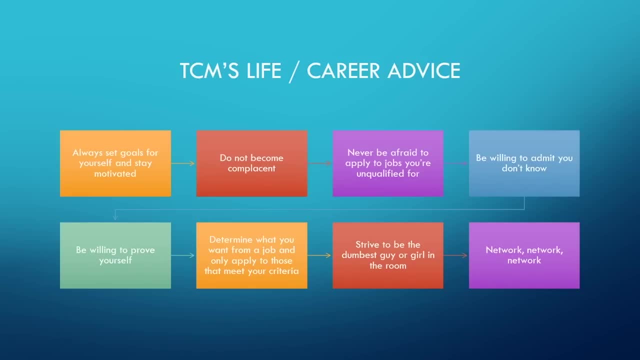 and you know, i had the opportunity to just sit there and i would go home and i would study, um, if there was downtime at work, i would study, you know, and i would just knock out certification after certification. um, and quickly i rose above my peers, right, because i was just putting in the work. 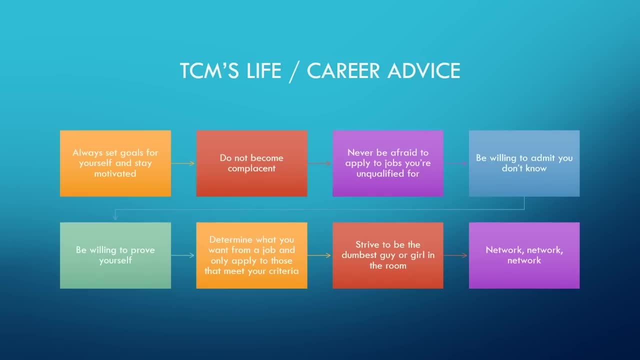 now. you will come across people in every single job that you work, no matter the level of the job. where there is complacency. you will find people who have been on help desk for 10 years. you will find people who have been in networking for 10 years, etc. it does not mean that it's bad. 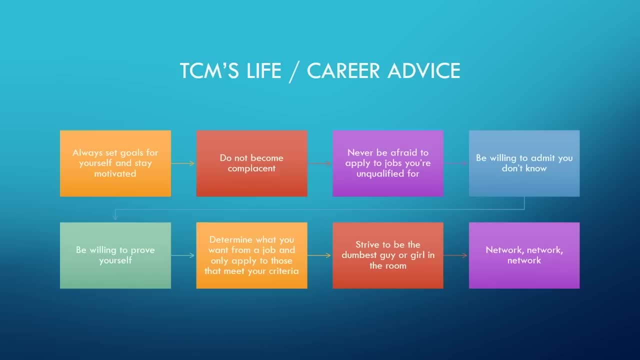 but it is just that if you want to be in information security, you shouldn't be complacent, right? you shouldn't be complacent, right? you don't have the ability to space sometimes to get started. You do not want to be that guy working the same job, getting the same pay. 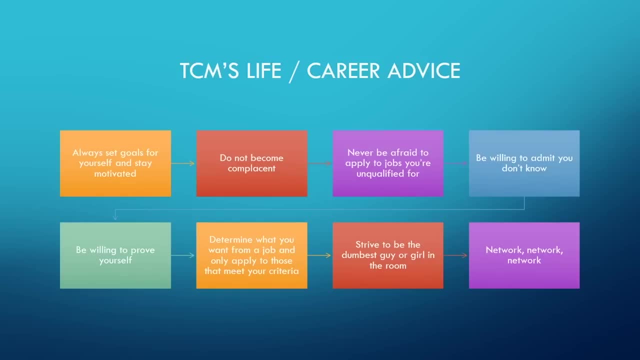 I know a guy that is making you know $50,000 a year. He's been in IT for over 10 years. He may be at like $60,000 now, But where I started at $40,000 and I was up to $140,000 in three years. 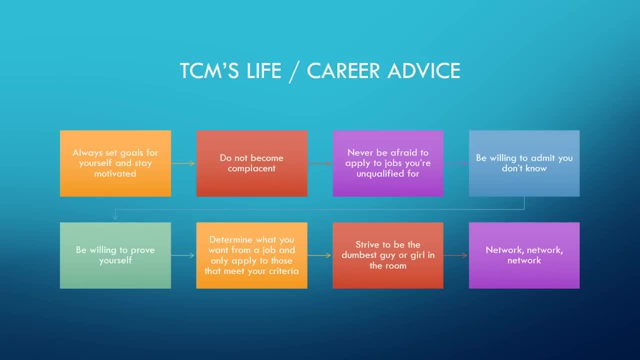 So I mean just, it's all motivation, A lot of it's luck, sure, But like you put in the time and you put in the effort, you're going to be rewarded. So you know, don't be that guy who's who's staying in the same position in the same job forever. 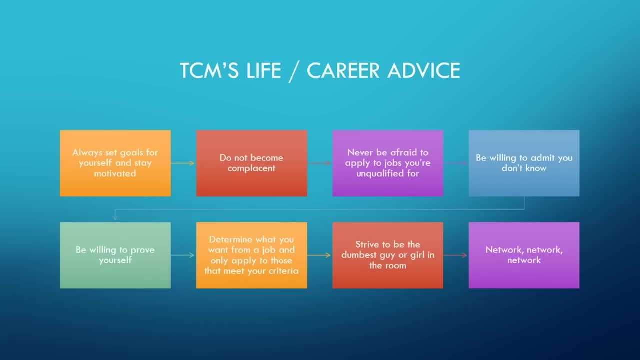 Always have that desire and that hunger to to move up. On top of that, you're going to want to never be afraid to apply to jobs that you are unqualified for. If I never applied to a job that I felt like I was unqualified for, I would never have a job because I was never technically qualified for anything. 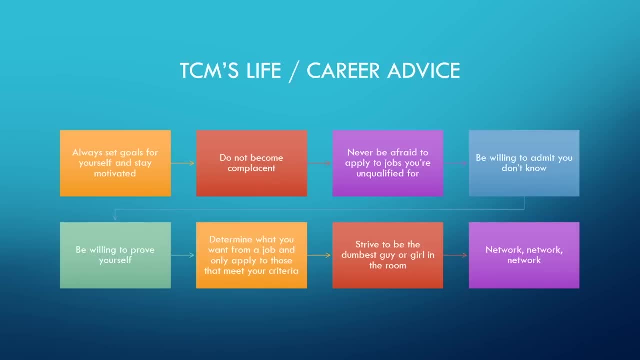 My first job with Help Desk. it was three years of experience, $50,000 a year was what they were offering. They wanted A plus, net plus, etc. I had no experience, nothing. I got into that interview and you know, I just told them like I don't know anything. but you know, I'm willing to learn. 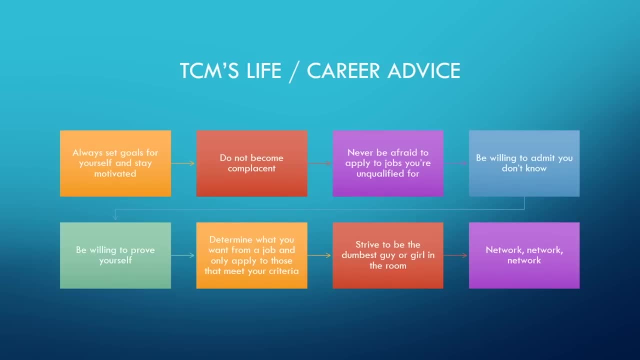 And those go into my next two concepts as well. Be willing to admit that you don't know, Especially in an interview. don't try to bullshit your way through things. Just say you know, I don't know, but I'll learn you know, or I don't know, but I'll prove myself. 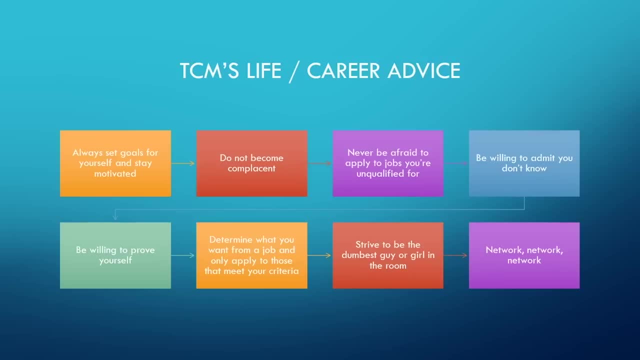 So you know, I went into that job and I said: look, I don't, I don't really know how to do this job. I don't got the credentials that you're looking for, But if you give me the opportunity, I will learn and I will prove myself. 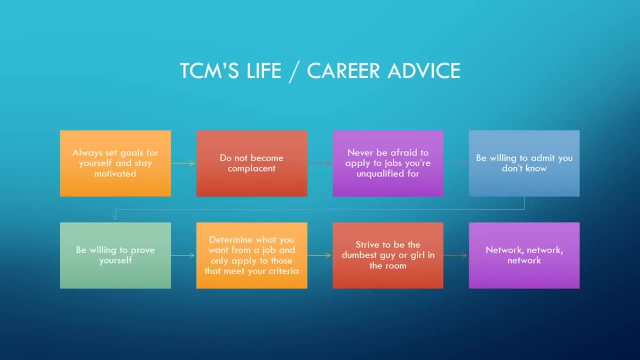 And you know, I even said, hey, I'll take less money just to come in and show you that I'm worth what it is. And I said, well, I don't know. And I said, well, I don't know. 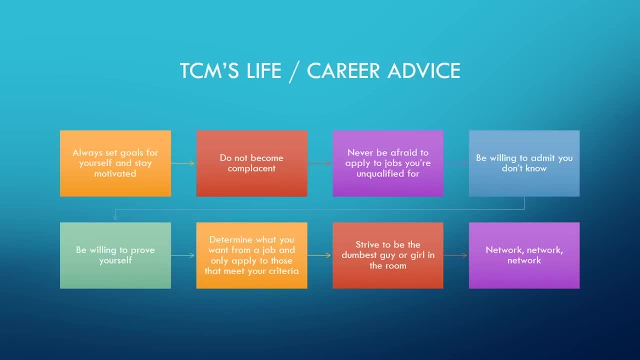 And I said, well, I don't know, And I did that. I came in at like 40, I think it was 42 or 44,000. And I was over 50,000 within a few months. Like they, they saw that I was putting the effort that I I really did deserve what I, you know. I said I would. 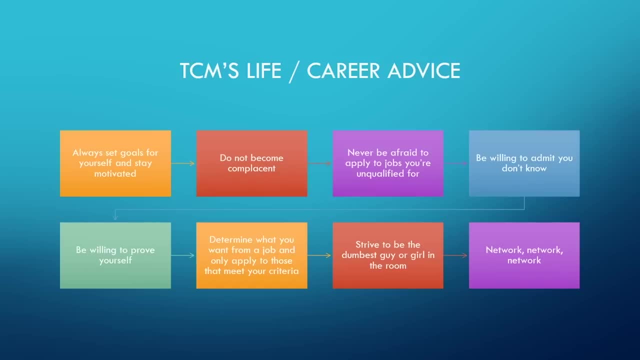 And I did that At the same time. with that, that job, and it falls into another thing. I feel like I feel like I outgrew it Right And it's part of that complacency: You don't want to be in the same place. 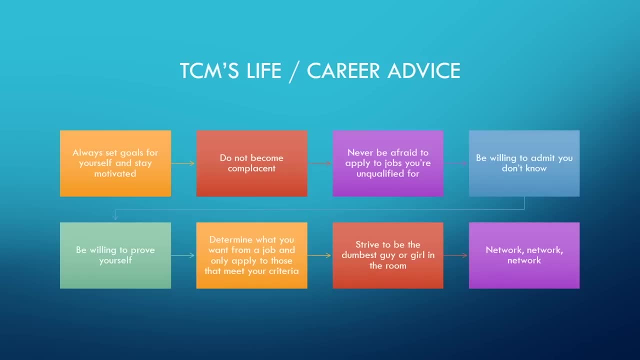 You don't want to be in the same job forever. You want to be able to move up and you want to get smarter, get better, And if you're outgrowing your job, you need to leave Right. So that falls into the next couple of bullet points here. 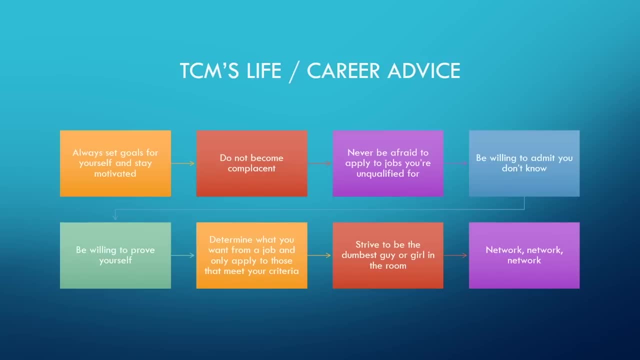 So first thing is you want to determine what you want from a job, Right, If you're unhappy, if you feel like you aren't the dumbest guy or girl in the room, which is the next tip as well, If you're not the dumbest guy or girl in the room, 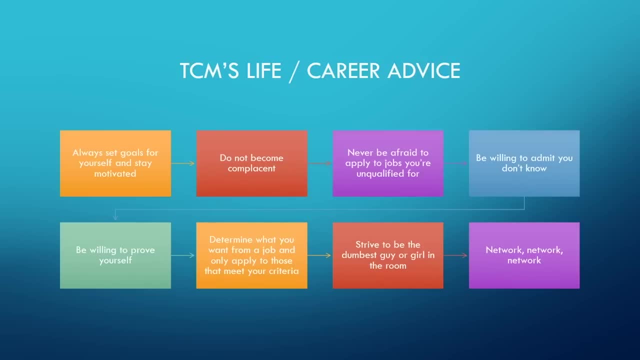 If you're not the dumbest guy or girl in the room anymore, it's probably time that you should leave and look for something else. So determine what you want from the current job you're in and from what the next job is, and only apply to those jobs that meet your criteria. 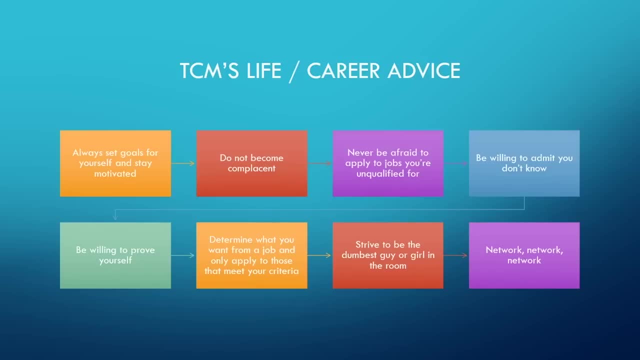 So I see a lot of people making the mistake of just applying to every single job. when they're, you know, like fresh LCPs, They'll apply to every single job that's out there, you know, just to hopefully land something. 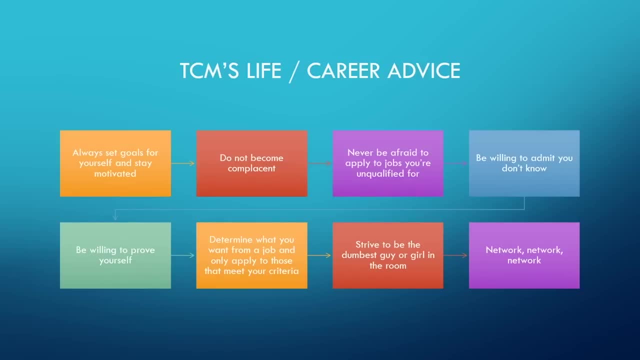 But you know, so many of them come back and like Five months and say, you know, I'm so unhappy at my job And it's like, well, you took the first thing that was offered to you. So you know, a job is a huge commitment. 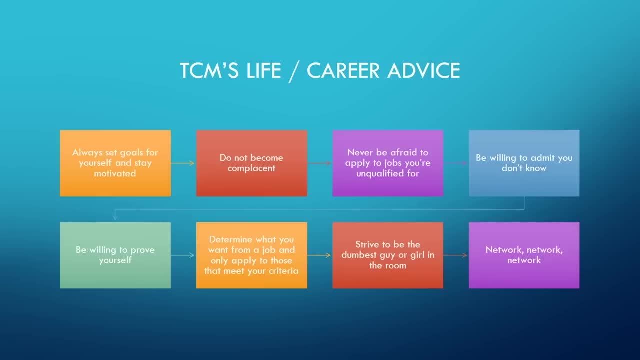 You should be picking your boss more than anything else. Right, You want a boss that's going to be good, that's not going to micromanage you, that's going to give you every opportunity to learn, to study, to go to conferences, to give talks, to have a blog, whatever. 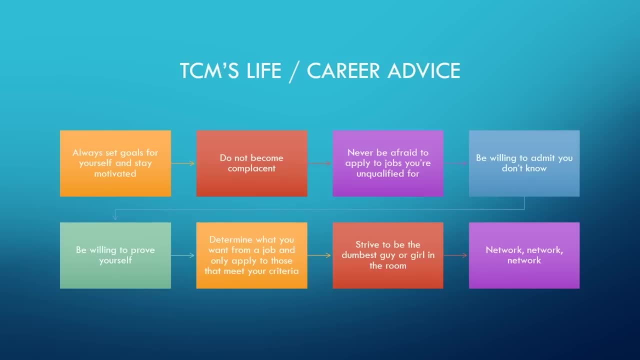 You want a boss that's going to encourage you to be better and continuously get better, So you need to suss that out during job interviews and make sure that everything's a fit. Don't just take the first job offer that comes to you. 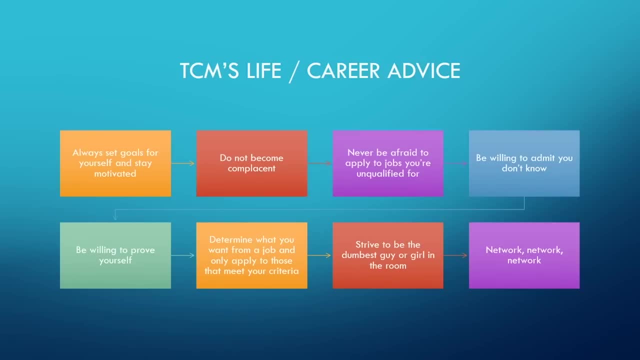 And it goes back into that point. Like I said, you want to strive to be the dumbest guy or girl in the room. If you are feeling you are in a opportunity where you're not, it is time to pack up and go somewhere else, especially in information security. 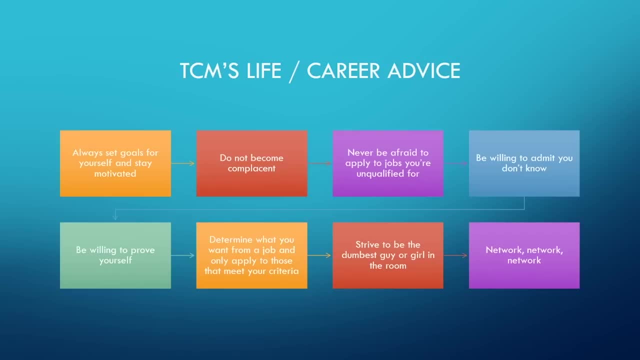 You want to be dumb all the time because there are so many smart people around you. So, last but not least, six years of business school that I went to. the one lesson they repeated over and, over and over and over is: network, network, network, right. 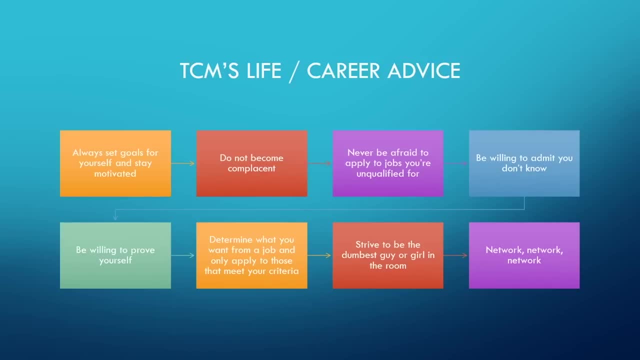 You never know who you're going to be nice to shoot a chat with. you know you might be on a job site one day talking to your future boss. you just don't know. So it's always good to put yourself out there to make connections, make friends. 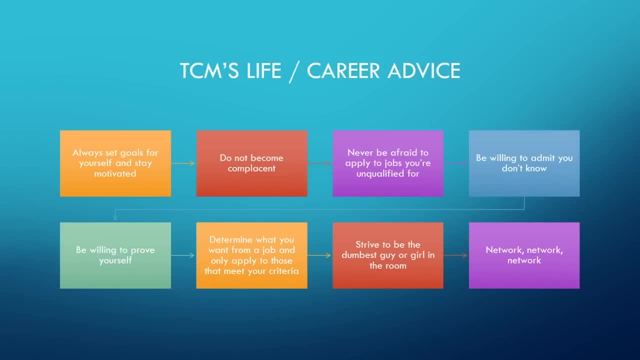 And just you know. let them know who you are, let them know that you're a talented individual, and someday it might just fall back into your lap. You're never going to know what dividends it's going to pay and how long it's going to take. 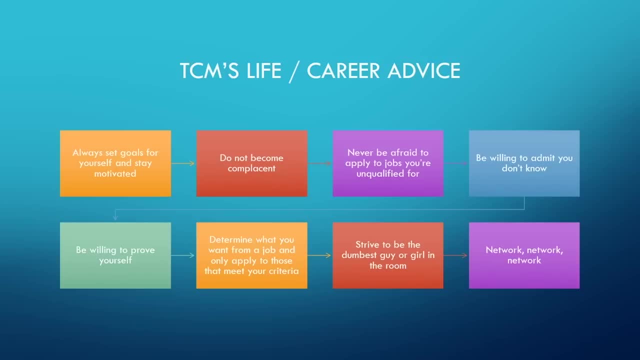 Sometimes you know you might not get a phone call for five years from somebody that you met, but you plant that seed and someday that seed is going to grow And it's all about building this network of people. I'm fully, fully attesting to that. 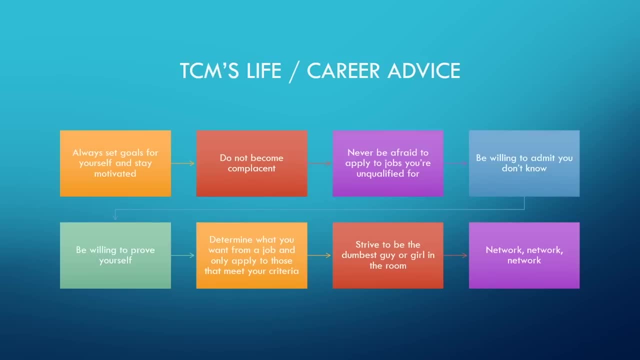 So like if you guys watch my first video on the entrepreneurship, like I quit my job without another job And somebody you know, somebody close to me, said: hey, like, hi, I see you're on the market. 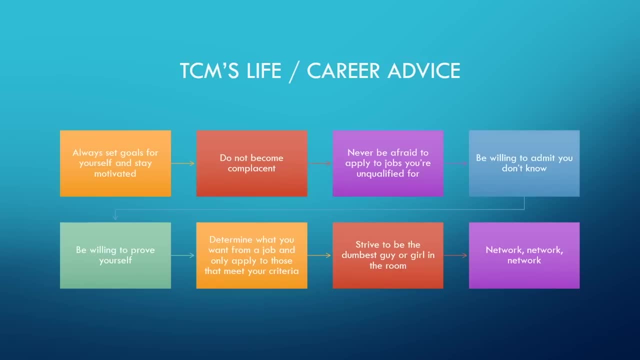 Do you want a job offer? And it was easy as that. There was no technical interview, There was no anything. It was like: hey, I know you're capable of doing the work. I've seen you work before. If you're interested in this job and you think it would be a good fit, I'd love to have you on the team. 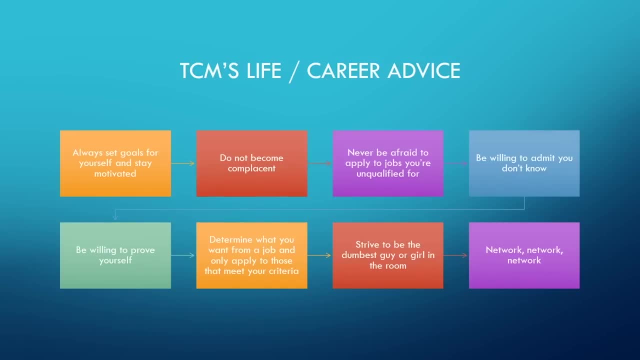 So it was that easy And you don't need to pick something else up. Not everything in your career as you go up is going to be, you know, super technical. this and that It's really comes down to who you know. 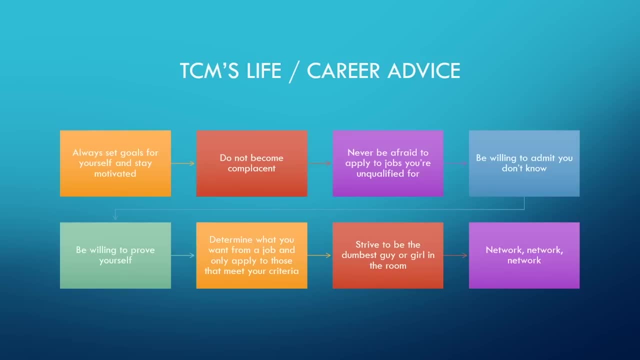 So make sure you're taking your time to network with people. Some people are saying business cards- Yeah, get good business cards, even if they're your own, your own personal business cards or your company's business cards. You know, just leave that impression, make that connection on LinkedIn and just strive to be a better person every single day. 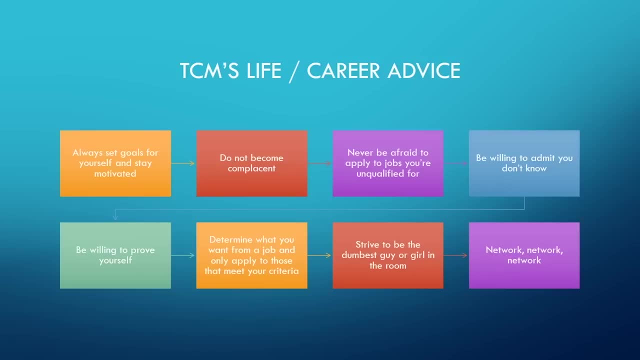 That is. that is it, guys, My career advice. That is that's it. I think we are. we are done, my people. I'm going to come back to the screen.